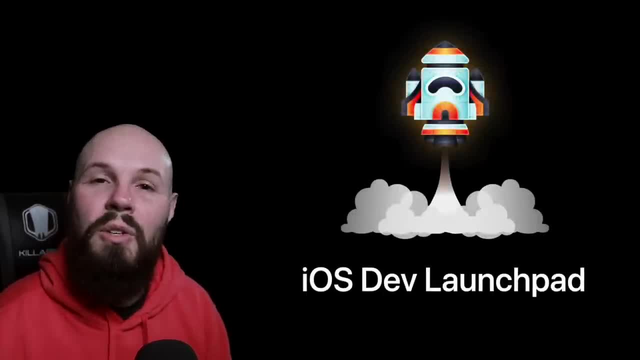 so that you could easily pass this off as somebody's very first steps into this world. right again, like you have a friend that says, hey, I want to learn that too. like this is the content you give them, and because this is meant for absolute beginners or those that are very early in their 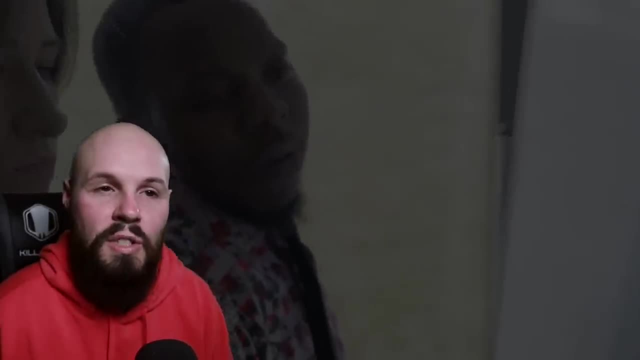 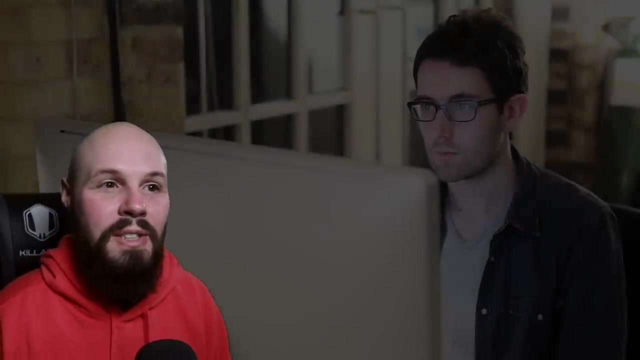 journey. I keep things at a high level. this course is all about just exposing you to this world and foundation, because this is the first step among many, but also because, again, I remember what that was like. this is how I learned: by doing online courses, YouTube videos. this is how I started my 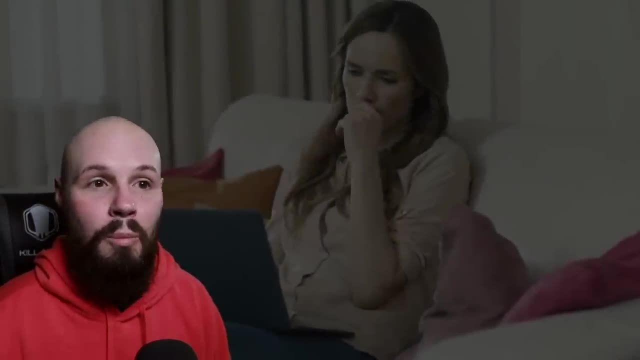 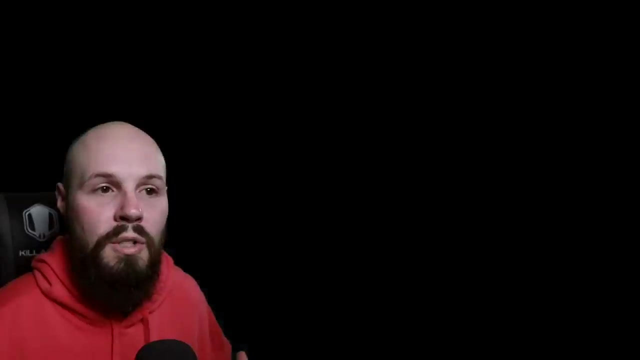 career, so I remember being completely overwhelmed. so there's a lot of topics that I could have gone deeper into and given you a ton of information, but what I'm trying to do with this course is walk a fine line between giving you enough information but not giving you too much to where you're. 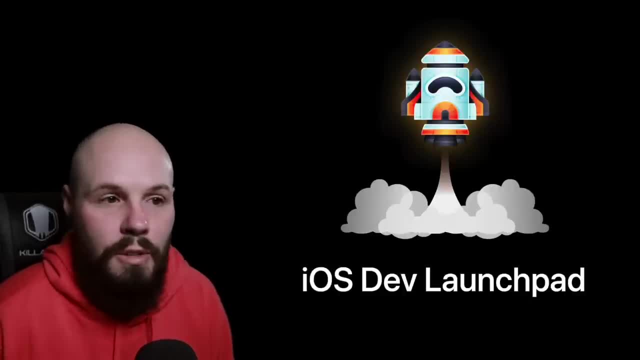 overwhelmed or it's confusing and you just you just kind of give up, right. so I'm trying to walk that balance. so I know some of you may say, oh, I wish you would have went deeper in that, or maybe in some topics I go too deep for you. but just know that, like I said, I'm 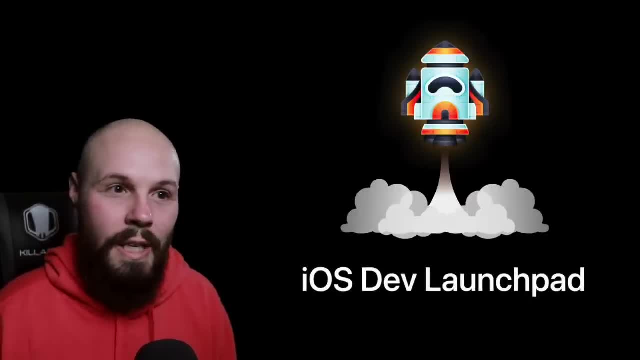 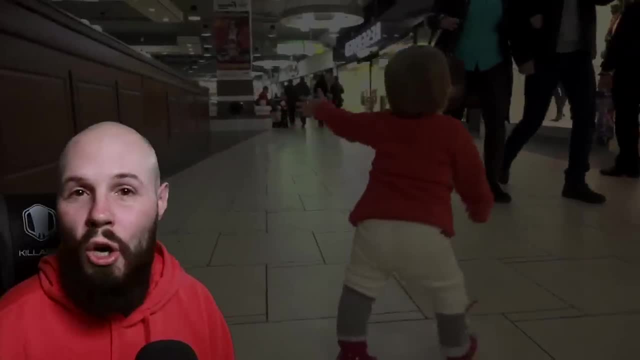 trying to walk that balance, because I know what it's like to be overwhelmed and sometimes getting all the information is more confusing than helpful because, like I said, this is step one on a long journey for you- most people that start from scratch- to get hired as a professional iOS developer. it. 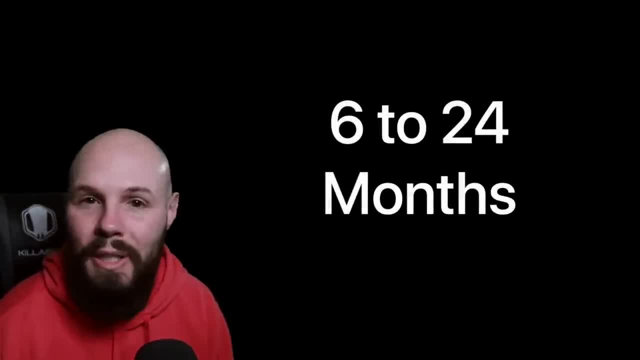 can take anywhere from six months to two years and everything in between. so don't think that you're gonna take this course and be ready like that's. this is not how it works right. this is a long journey: at least six months of hardcore learning, likely even longer, so I just want to set those expectations. another: 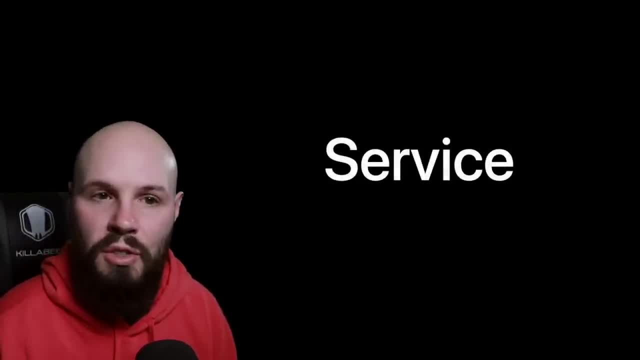 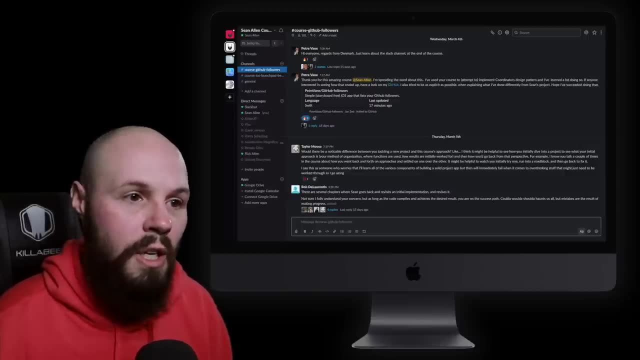 thing I wanted to be sure to include with this course is good service. so I've created a slack channel. that's for all my courses, right, but each course has their own individual room. but this is a slack channel that you can join and go in and get real-time help, not only for me, but from 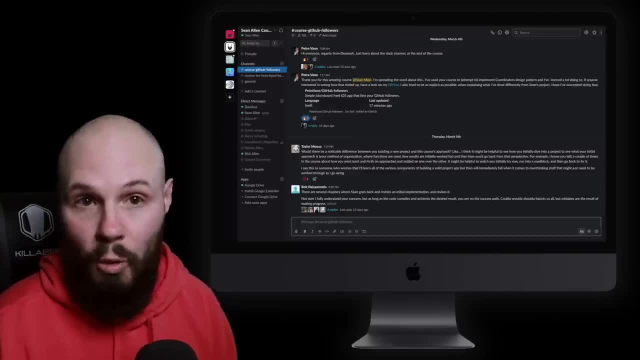 all of my courses, right, but each course has their own individual room. but this is a slack channel that you can join and go in and get real time help, not only for me but from other students. like I said, that slack channel is for all my courses, so you're. 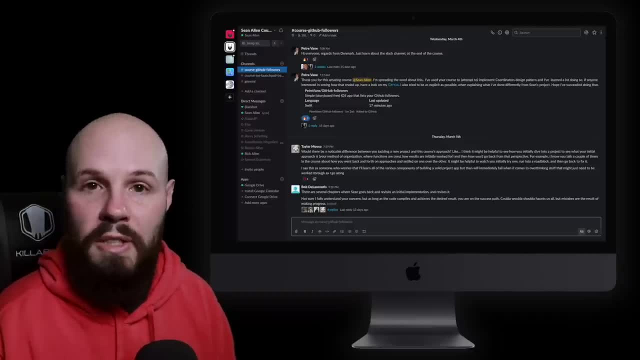 you're not just gonna get beginner developers in there, you're gonna get more experienced developers in there as well, and what I've seen so far is that people have been very helpful in that slack channel, and I'm very thankful for that because, as you know, thousands of students come into these courses. I just 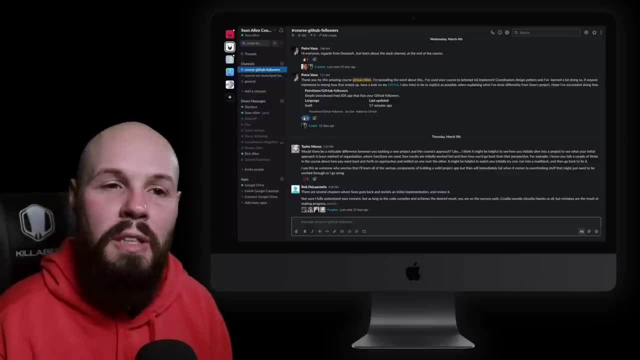 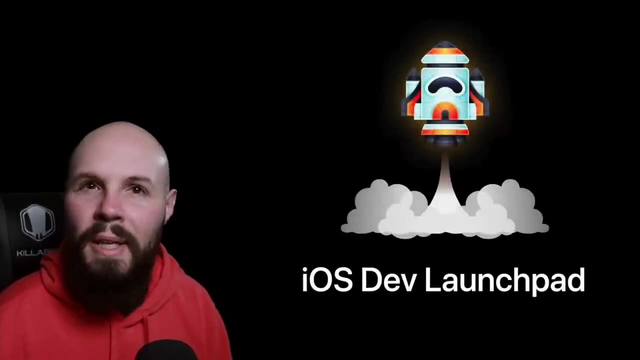 can't answer everybody's questions. so we're trying to build a good community to help each other out in that slack channel, so be sure to join that. so let's finish up going over the structure of the course. so for about the first 40 to 50 percent of it, we're gonna go through the structure of the course. so for about 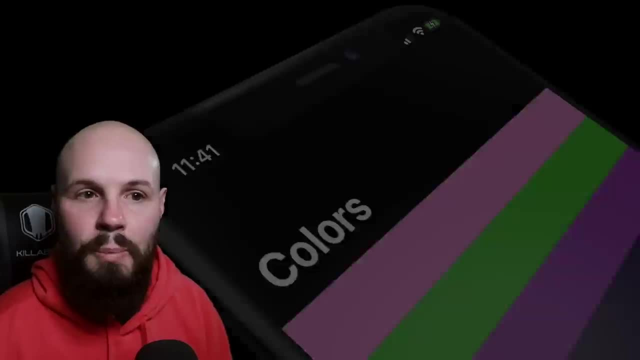 50 percent of it. we're gonna go through the structure of the course. so for about be going over the basics of the Swift language, then we move on into building a. be going over the basics of the Swift language, then we move on into building a couple of, you know, basic beginner apps. we're also gonna break down one of these. 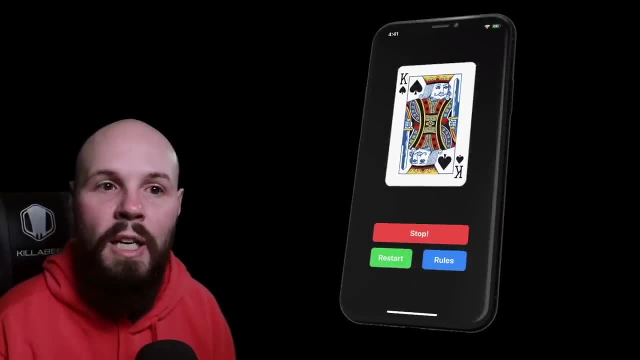 couple of you know, basic beginner apps. we're also gonna break down one of these apps where we build it the first time using storyboard and interface builder. apps where we build it the first time using storyboard and interface builder and the second time we're gonna build it all programmatic UI. so you get a little. 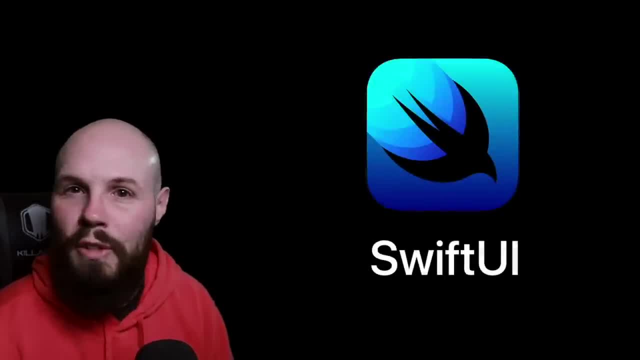 and the second time we're gonna build it all programmatic UI. so you get a little taste of both, and I also have a little Swift UI preview section talking about taste of both, and I also have a little Swift UI preview section talking about what it is why this is a very different way of doing things. and then we build. 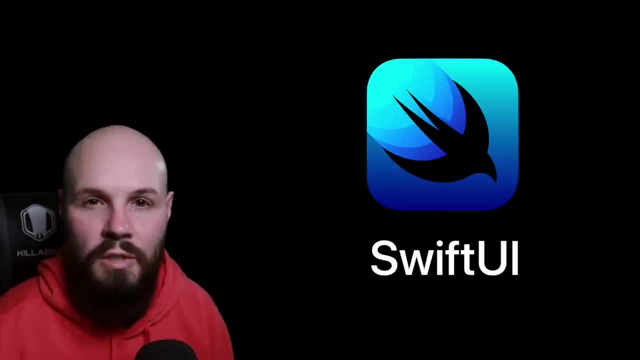 what it is, why this is a very different way of doing things. and then we build like a little sample screen with it, but like a little sample screen with it, but like a little sample screen with it, but the reason this whole course doesn't, the reason this whole course doesn't- 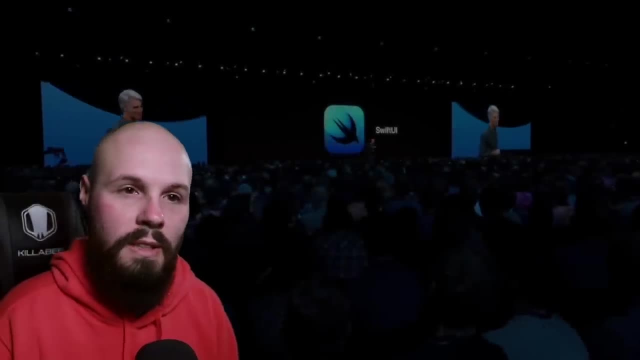 the reason this whole course doesn't focus on Swift UI is because you know it. focus on Swift UI is because you know it. focus on Swift UI is because you know it was just announced in summer of 2019. was just announced in summer of 2019. 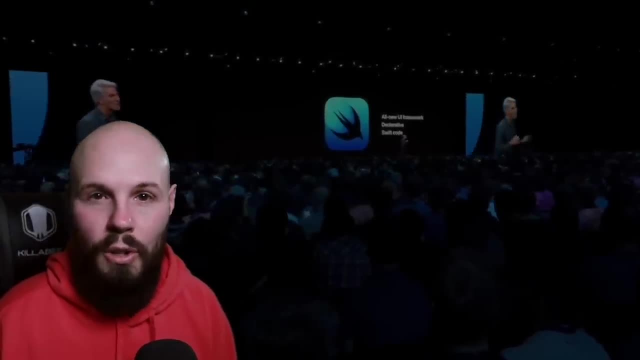 was just announced: in summer of 2019. it's still very early. it's gonna take a. it's still very early. it's gonna take a. it's still very early. it's gonna take a long time for you know major apps to long time for you know major apps to. 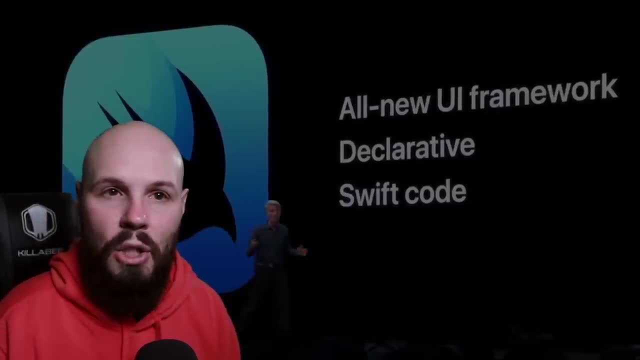 long time for, you know, major apps to adopt it. it will have its day, but it's adopt it. it will have its day, but it's adopt. it will have its day, but it's still very early. so again, if you're still very early. so again if you're. 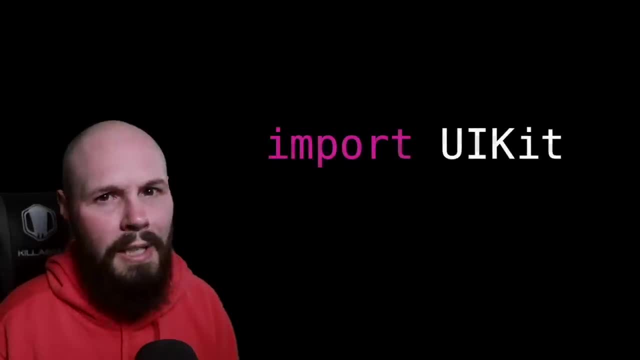 still very early. so again, if you're trying to get a job in the next six, trying to get a job in the next six, trying to get a job in the next six months to two years, UI kit is still. months to two years, UI kit is still. 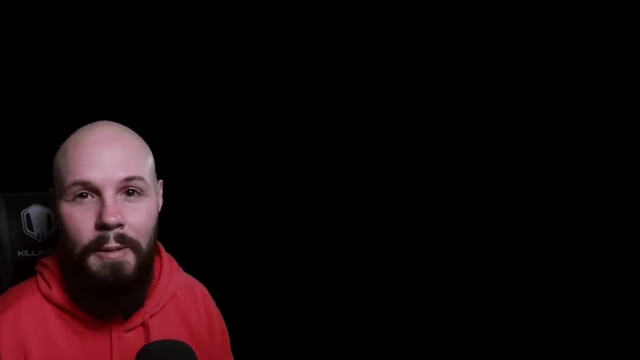 months to two years, UI kit is still gonna be very, very dominant. but we give gonna be very, very dominant. but we give gonna be very, very dominant. but we give you a little taste of Swift UI here and you a little taste of Swift UI here and you a little taste of Swift UI here, and then we move on to kind of like the 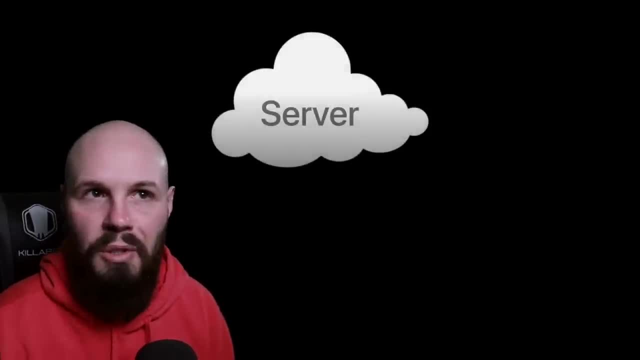 then we move on to kind of like the. then we move on to kind of like the general programming knowledge section- general programming knowledge section- general programming knowledge section. talking about you know how apps work. talking about you know how apps work. talking about you know how apps work, that, the server, the client, what is an? 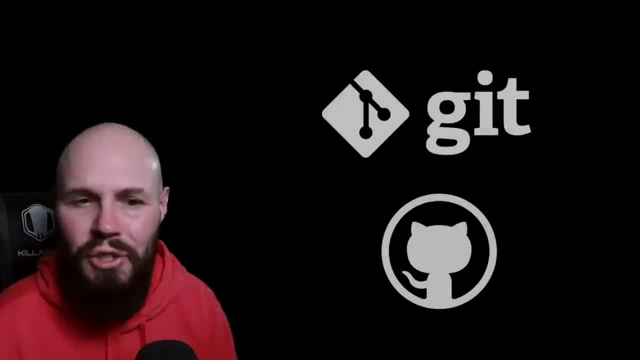 that the server, the client. what is an that the server, the client. what is an API? what are third-party libraries? how API? what are third-party libraries? how API? what are third-party libraries? how does version control work we talk about? does version control work? we talk about. 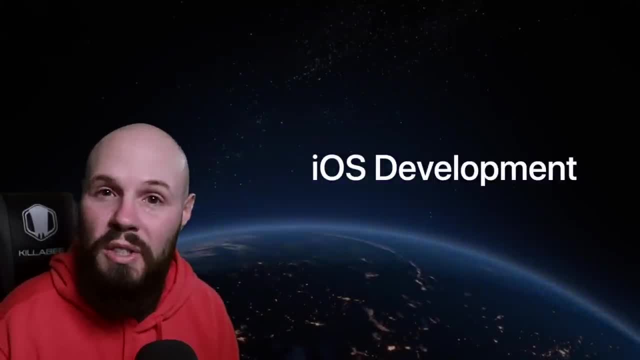 does version control work? we talk about different career paths, and then I start different career paths, and then I start different career paths and then I start recommending some resources again, recommending some resources, again recommending some resources again: podcasts, blogs, websites, videos, books, podcasts, blogs, websites, videos, books, podcasts, blogs, websites, videos, books. again, I want to set you up for future. 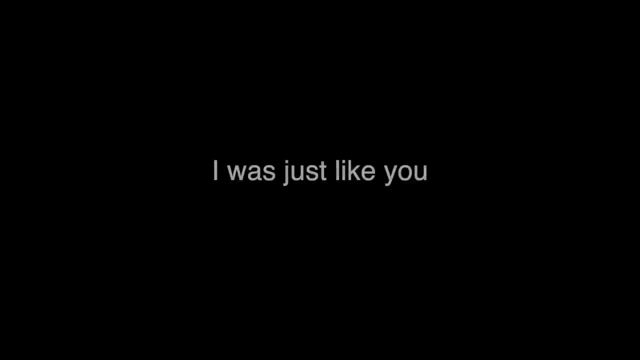 again, I want to set you up for future. again, I want to set you up for future learning, because this is the very first learning, because this is the very first learning, because this is the very first step in your journey, step in your journey, step in your journey. a little over five years ago, I was just 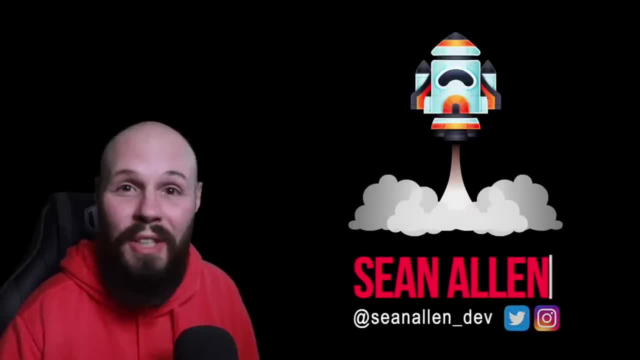 a little over five years ago- I was just a little over five years ago- I was just like you. I was trying to learn how to like you. I was trying to learn how to like you. I was trying to learn how to code just by watching online videos. 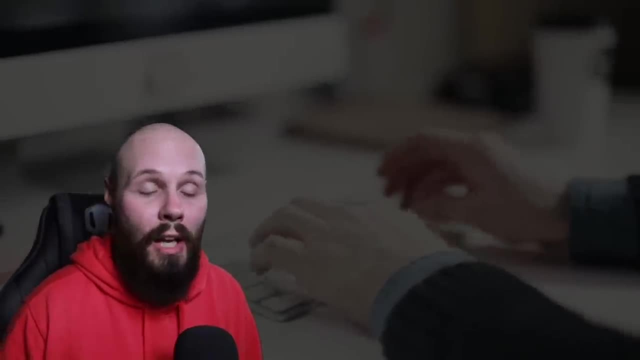 code just by watching online videos code just by watching online videos, taking online courses, and I wrote my taking online courses and I wrote my taking online courses and I wrote my first line of code at 32 years old. had. first line of code at 32 years old, had. 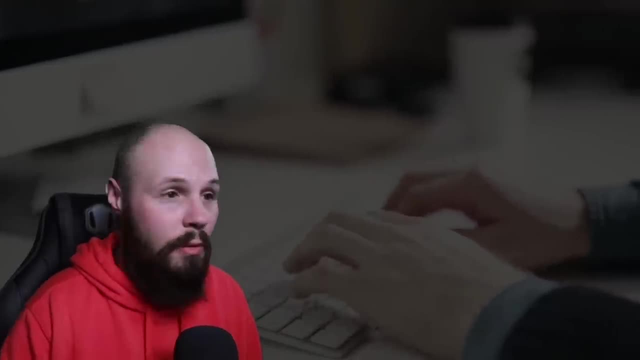 first line of code at 32 years old, had no prior programming experience- just no prior programming experience, just no prior programming experience. just wanted to do a career change and was wanted to do a career change and was wanted to do a career change and was interested in this and I wanted to. 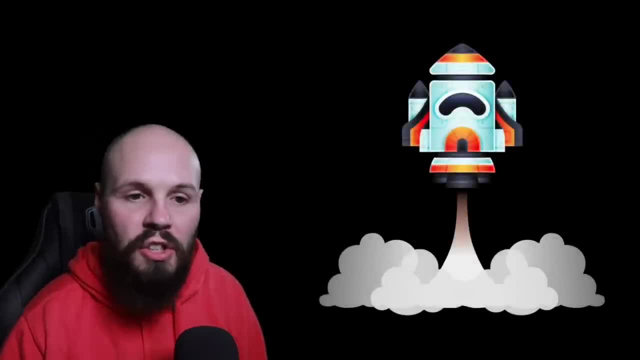 interested in this and I wanted to interested in this and I wanted to create a quick video in this beginner. create a quick video in this beginner. create a quick video in this beginner course. going over my story just to show course. going over my story, just to show. 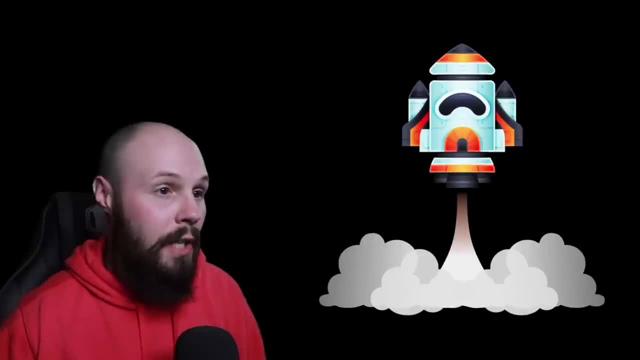 course, going over my story, just to show that, like again, I didn't start coding that. like again, I didn't start coding that. like again, I didn't start coding till I was 32, I had no prior programming. till I was 32, I had no prior programming. till I was 32. I had no prior programming experience and I've done very well for experience. and I've done very well for experience and I've done very well for myself and I don't say that to brag myself and I don't say that to brag. 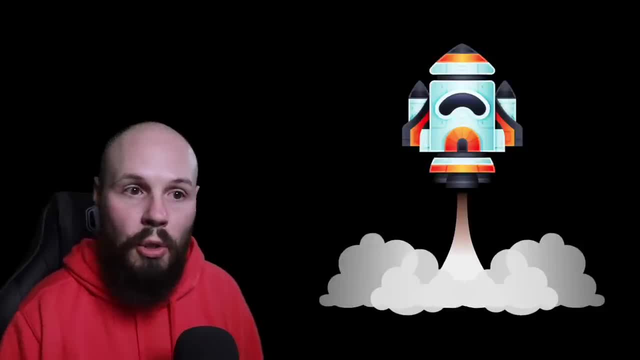 myself, and I don't say that to brag again. the point of this video is to show again. the point of this video is to show again. the point of this video is to show you you know somebody that was in your. you know somebody that was in your. 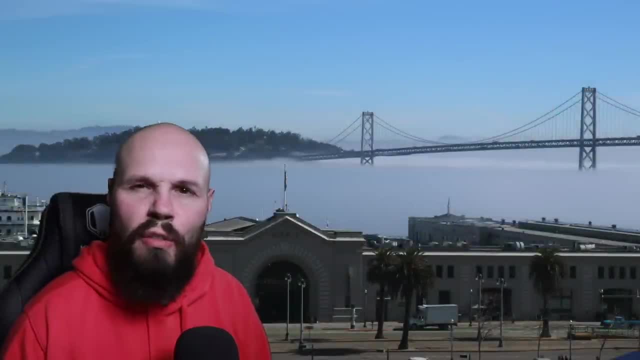 you know somebody that was in your shoes and that has done it so like I said shoes, and that has done it so like I said shoes, and that has done it. so, like I said, I've been an iOS engineer for about. I've been an iOS engineer for about. 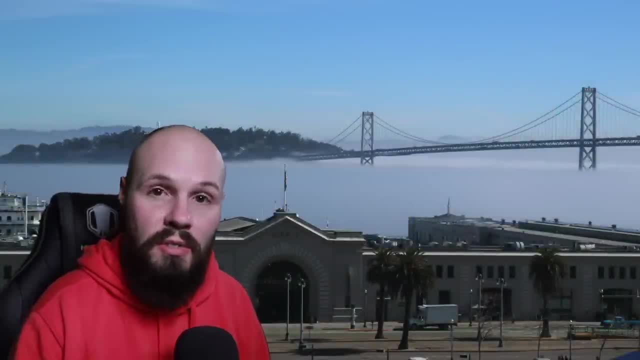 I've been an iOS engineer for about five years now, just about all of which was five years now, just about all of which was five years now, just about all of which was spent in San Francisco in Silicon, spent in San Francisco in Silicon, spent in San Francisco in Silicon Valley. how I got interested in all this. 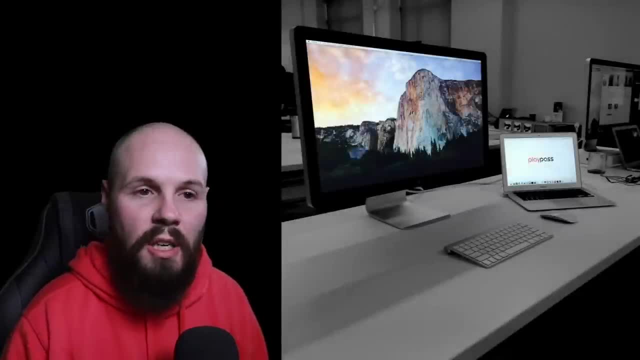 Valley. how I got interested in all this Valley. how I got interested in all this is: I was working for a startup out there is. I was working for a startup out there is. I was working for a startup out there as a growth lead sales type stuff and I 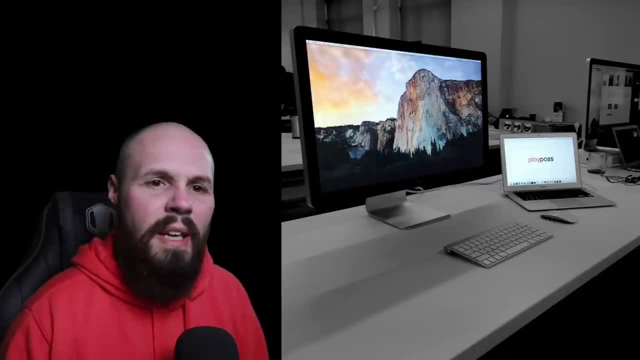 as a growth lead sales type stuff and I as a growth lead sales type stuff, and I just became friends with our engineers. just became friends with our engineers, just became friends with our engineers because it was a small team, small. because it was a small team, small because it was a small team, small startup. and I started asking questions. 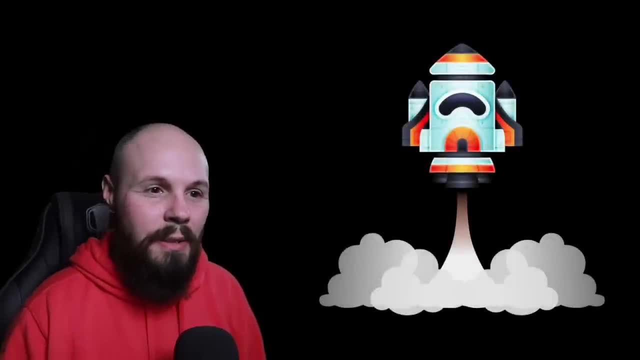 startup and I started asking questions startup and I started asking questions about what they were doing and just about what they were doing and just about what they were doing and just about coding in general and to be honest about coding in general and to be honest about coding in general and to be honest with you- and I hope this doesn't come- with you and I hope this doesn't come with you, and I hope this doesn't come off as arrogant, but after getting to off as arrogant, but after getting to off as arrogant, but after getting to know them and seeing what they did, I was know them and seeing what they did, I was. 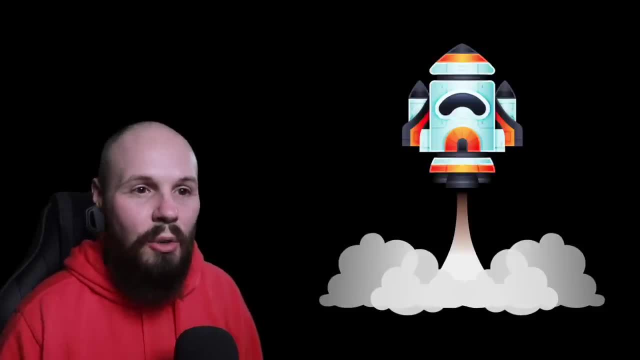 know them and seeing what they did, I was like I'm just as smart as them. there's like I'm just as smart as them. there's like I'm just as smart as them. there's no reason I can't do that, so I started. no reason I can't do that, so I started. 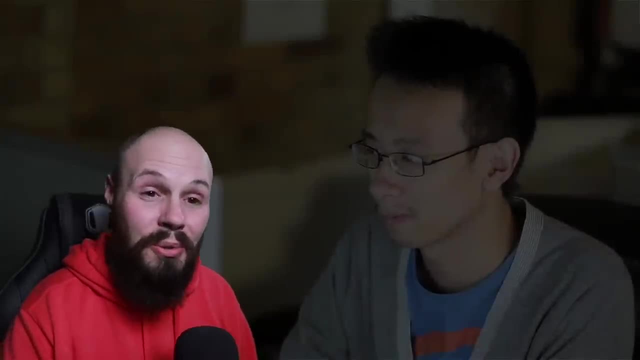 no reason I can't do that. so I started exploring, started googling doing online exploring. started googling doing online exploring. started googling doing online videos YouTube. you know buying online videos YouTube. you know buying online videos YouTube. you know buying online courses. again, I was exactly where you. 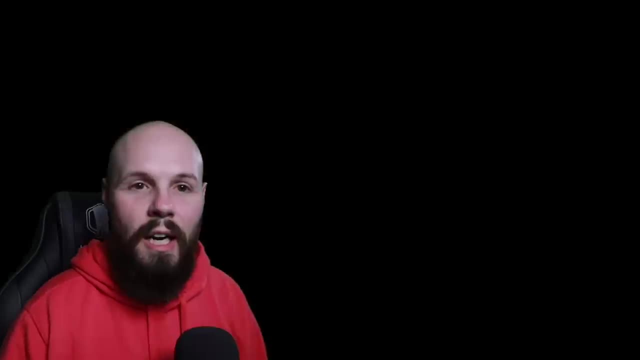 courses again. I was exactly where you courses again. I was exactly where you are right now. so when I started learning are right now. so when I started learning are right now. so when I started learning, it was early 2015, by summer of 2015, I. 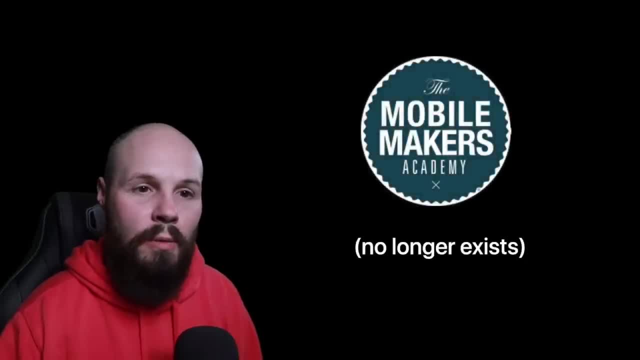 it was early 2015, by summer of 2015. I- it was early 2015. by summer of 2015, I did an iOS developer boot camp. now, I did an iOS developer boot camp now. I did an iOS developer boot camp now. I know what you may be thinking. well, you, know what you may be thinking. well, you know what you may be thinking. well, you know, boot camp is great. that's what know. boot camp is great. that's what know. boot camp is great. that's what. that's what gave you that head start, but that's what gave you that head start. but 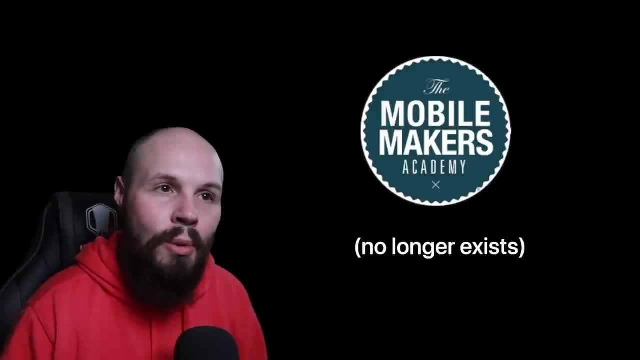 that's what gave you that head start. but now that I've done the boot camp, and now that I've done the boot camp, and now that I've done the boot camp, and I've, you know, created tutorials, like you, I've, you know, created tutorials, like you. 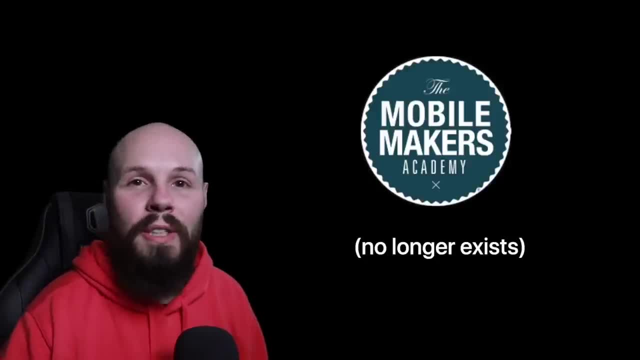 I've, you know, created tutorials. like you, don't you just learn the very basics in? don't you just learn the very basics in? don't you just learn the very basics in the boot camp? like everything I learned the boot camp. like everything I learned the boot camp. like everything I learned in the boot camp is in like super. 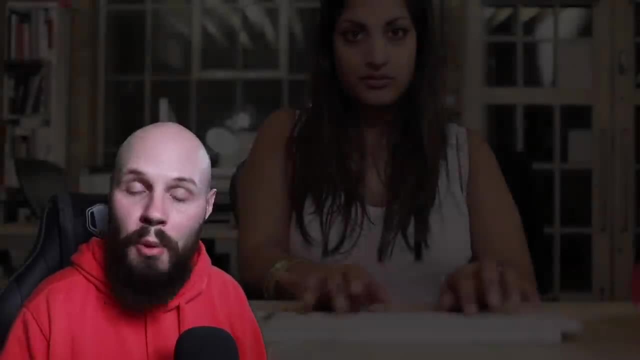 in the boot camp is in like super in the boot camp is in like super. beginner online YouTube videos- right the beginner online YouTube videos. right the beginner online YouTube videos- right. the benefit of the boot camp for me was benefit of the boot camp for me was. benefit of the boot camp for me was forcing myself to work on it for eight. 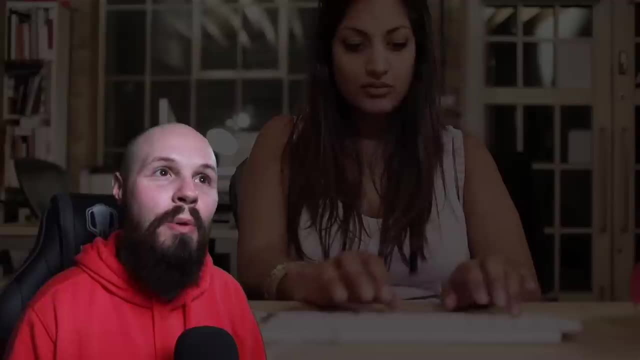 forcing myself to work on it for eight, forcing myself to work on it for eight hours a day. right because you got to be hours a day. right because you got to be hours a day. right because you got to be there for two months. eight hours, so that 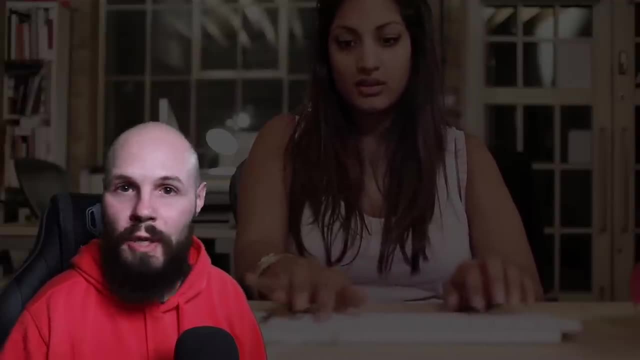 there for two months, eight hours. so that there for two months, eight hours. so that was the huge benefit of the boot camp. was the huge benefit of the boot camp? was the huge benefit of the boot camp? not I got crazy good knowledge or crazy. not I got crazy good knowledge or crazy. 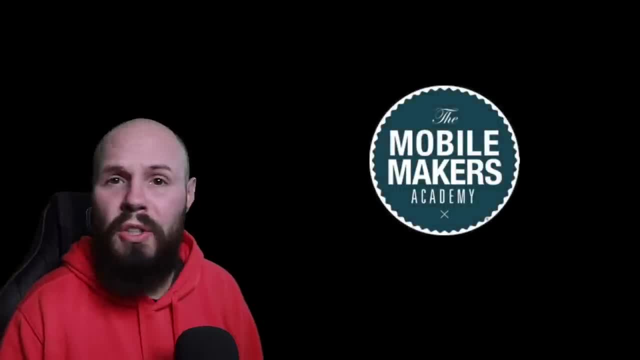 not I got crazy good knowledge or crazy good teachers. it just forced me to do it good teachers. it just forced me to do it good teachers. it just forced me to do it. but my boot camp was a good experience, I. but my boot camp was a good experience, I. 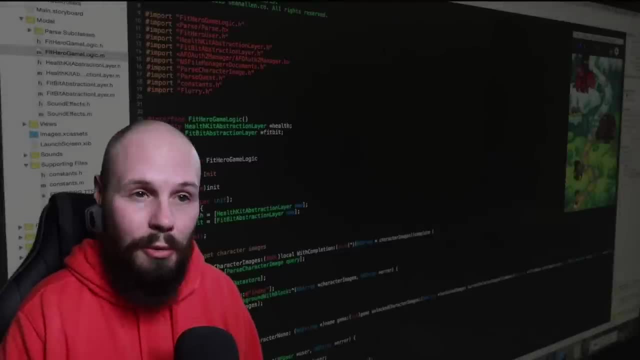 but my boot camp was a good experience. I like the people I graduated with. we like the people I graduated with. we like the people I graduated with. we ended up building an app called fit hero, ended up building an app called fit hero, ended up building an app called fit hero, which I really really like. you're. which I really really like. you're, which I really really like. you're seeing some screens of that. thought it seeing some screens of that. thought it seeing some screens of that. thought it was pretty cool in about a month and a was pretty cool in about a month and a. 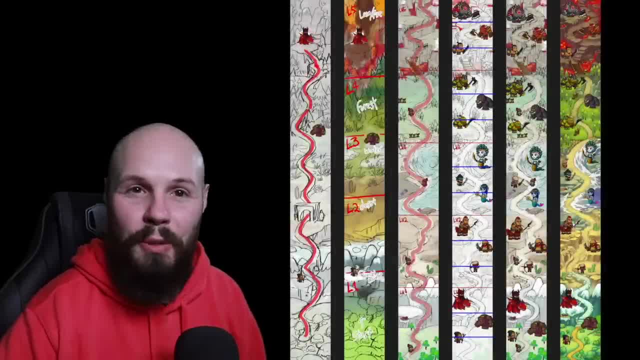 was pretty cool. in about a month and a half after the boot camp, I got hired. at half after the boot camp I got hired at half after the boot camp I got hired at my first real iOS developer job. so now my first real iOS developer job. so now, 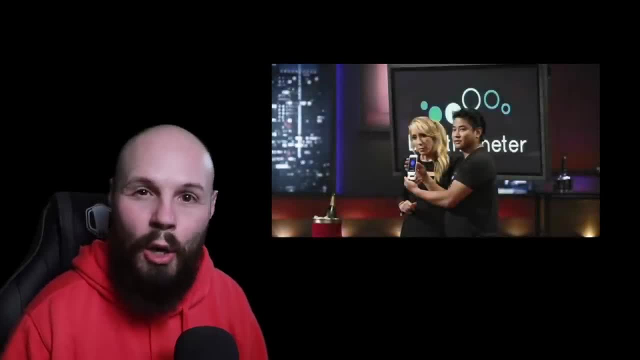 my first real iOS developer job. so now we're talking November 2015 at a company. we're talking November 2015 at a company. we're talking November 2015 at a company called breathometer. they were on shark called breathometer. they were on shark. 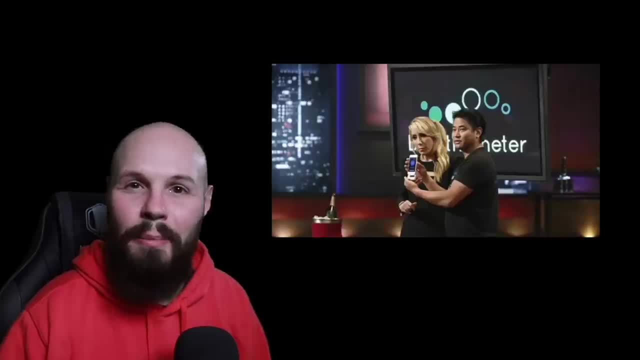 called breathometer. they were on shark tank. they were the first company to get tank. they were the first company to get tank. they were the first company to get all five sharks to invest. I think they all five sharks to invest. I think they all five sharks to invest. I think they got like a million dollar investment. 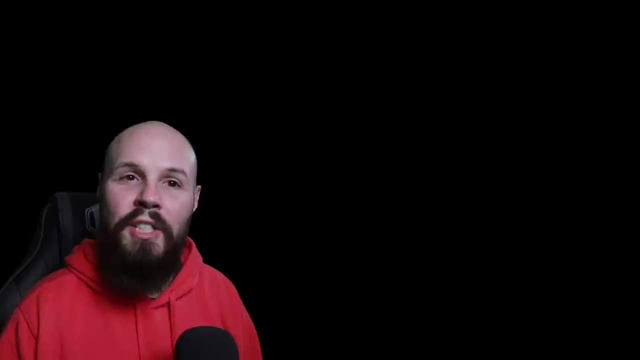 got like a million dollar investment. got like a million dollar investment. this was back in 2013. that was a pretty. this was back in 2013, that was a pretty. this was back in 2013. that was a pretty big deal for the time, but I got that job. 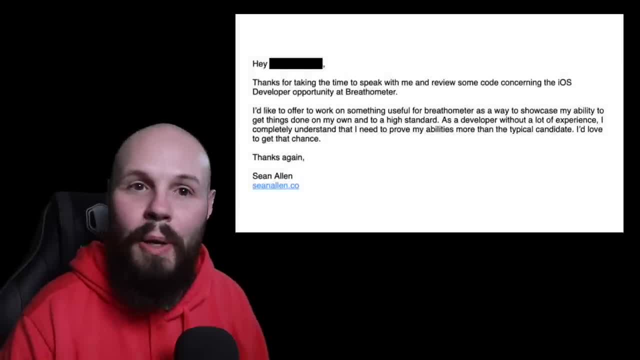 big deal for the time, but I got that job. big deal for the time, but I got that job initiative. I emailed them and said, hey, initiative. I emailed them and said hey, initiative. I emailed them and said, hey, look, I know I didn't do well on that do. look, I know I didn't do well on that do. look, I know I didn't do well on that. do you have a take-home project that I could? you have a take-home project that I could? you have a take-home project that I could do something I could work on that I? 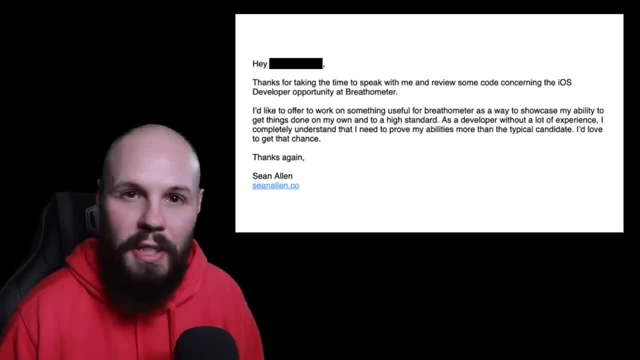 do something I could work on that. I do something I could work on that I can really showcase my skills. because I can really showcase my skills, because I can really showcase my skills, because I know as somebody without a CS degree and know as somebody without a CS degree and 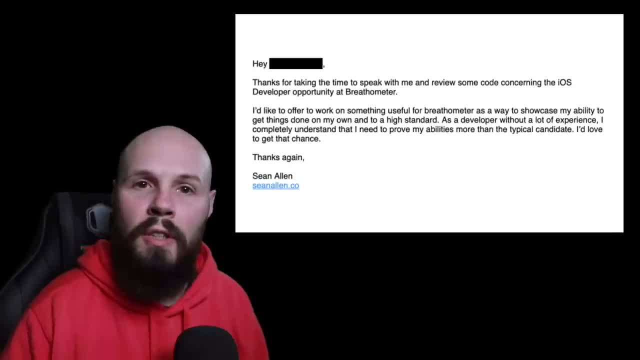 know, as somebody without a CS degree and just a boot camp grad, I know I have to just a boot camp grad. I know I have to just a boot camp grad. I know I have to prove myself even more, so I would love prove myself even more, so I would love. 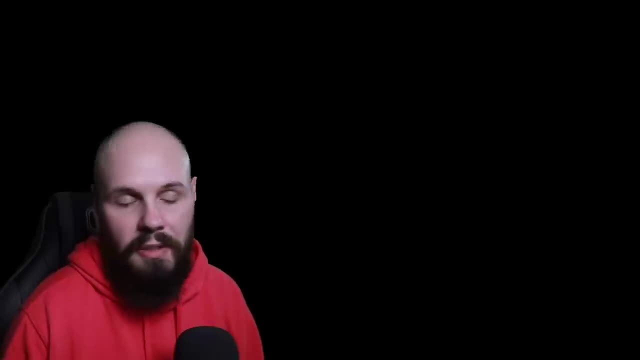 prove myself even more. so I would love to do a take-home project and show you to do a take-home project and show you to do a take-home project and show you what I can do. that was basically the. what I can do. that was basically the. 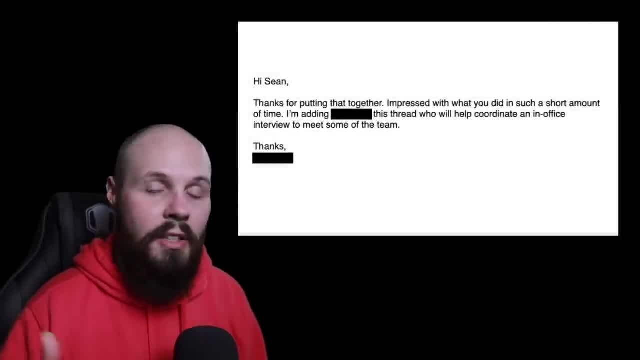 what I can do. that was basically the email and they said sure and long story email. and they said sure and long story email and they said sure and long story short. I did the project, they loved it short. I did the project, they loved it short. I did the project, they loved it and I got hired. so I guess the tip there. 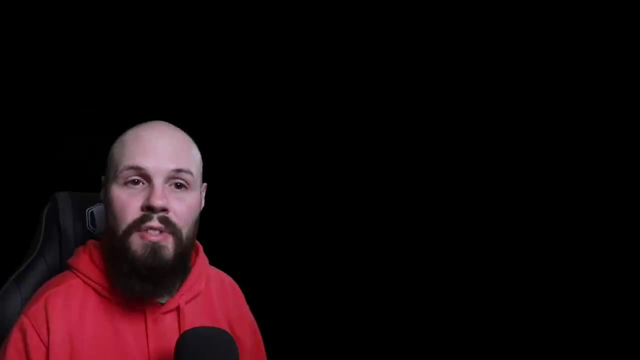 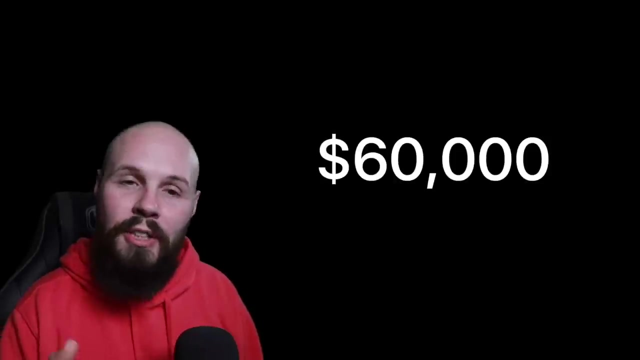 and I got hired. so I guess the tip there and I got hired, so I guess the tip there is: don't be afraid to show some is don't be afraid to show some is don't be afraid to show some of the things that you can do. and I took it. 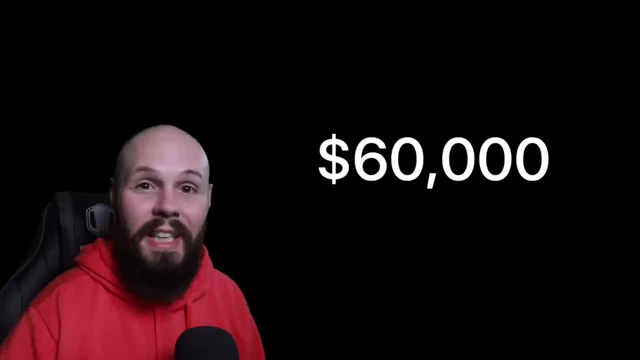 of the things that you can do and I took it of the things that you can do. and I took it because again I had applied to 60, because again I had applied to 60, because again I had applied to 60 companies. I wasn't getting any jobs, like companies: I wasn't getting any jobs. like companies: I wasn't getting any jobs. like it was rough getting that first job, so I: it was rough getting that first job, so I: it was rough getting that first job, so I was like I just need somebody to take a. 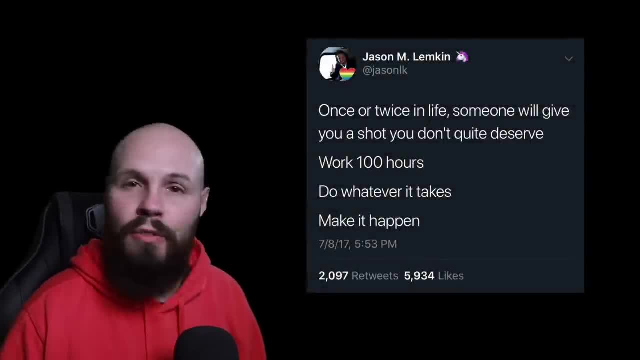 was like I just need somebody to take a was like I just need somebody to take a chance on me. I know I can get in there. chance on me. I know I can get in there. chance on me, I know I can get in there. you know, prove myself and I'll ask for a. you know, prove myself and I'll ask for a. you know, prove myself and I'll ask for a raise in like six months. like that was raise in like six months. like that was raise in like six months. like that was my plan. like because I knew I would get. my plan, like because I knew I would get my plan, like because I knew I would get in there and perform like I'd confidence in there. and perform like I'd confidence in there and perform like I'd confidence in myself, and within a month and a half, in myself and within a month and a half in myself and within a month and a half of working there, my VP of software, my of working there, my VP of software, my of working there, my VP of software, my boss kind of pulled me aside and was boss kind of pulled me aside and was. boss kind of pulled me aside and was: like I'm working on a race for you, like like I'm working on a race for you, like like I'm working on a race for you, like you deserve it, we need to pay you the. you deserve it, we need to pay you the. 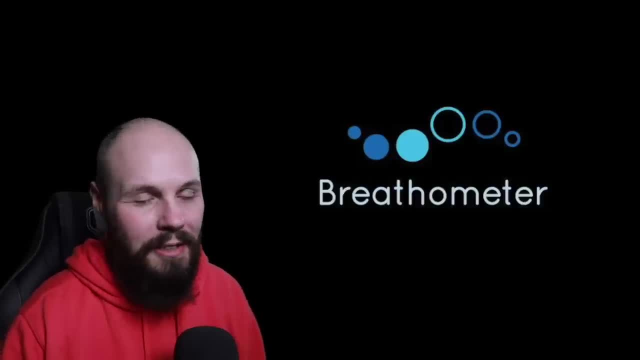 you deserve it. we need to pay you the just market rate. it wasn't like I was just market rate. it wasn't like I was just market rate. it wasn't like I was getting superstar money, but just market getting superstar money, but just market getting superstar money, but just market rate, because 60,000 was not market rate. rate because 60,000 was not market rate rate, because 60,000 was not market rate. long story short like a series: a funding. long story short like a series, a funding. long story short like a series, a funding, like delayed it and delayed it and. 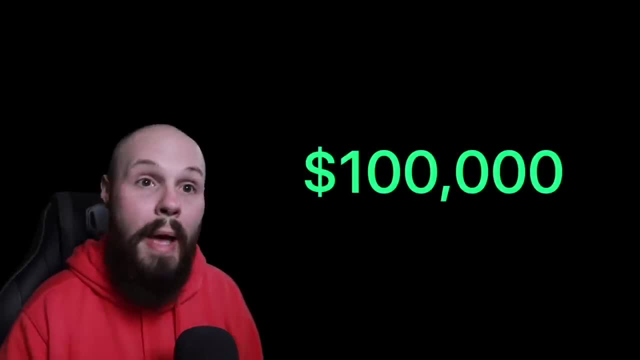 like delayed it and delayed it. and like, delayed it and delayed it and delayed it. um, anyway, I ended up getting delayed it. um, anyway, I ended up getting delayed it. um, anyway, I ended up getting 100k by May of 2016.. so I'm six months. 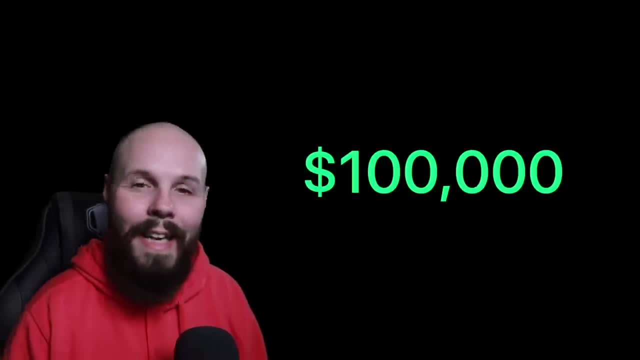 100k by May of 2016.. so I'm six months: 100k by May of 2016.. so I'm six months in to my first ever job and I crossed in to my first ever job and I crossed in to my first ever job and I crossed the six-figure mark and again I don't. the six-figure mark. and again, I don't the six-figure mark. and again I don't say this to brag. I say this to just let say this to brag. I say this to just let say this to brag. I say this to just let you know what's possible. so I worked at. you know what's possible, so I worked at. you know what's possible, so I worked at Brathometer for about a year and a half Brathometer for about a year and a half Brathometer for about a year and a half, and then I left there to start. 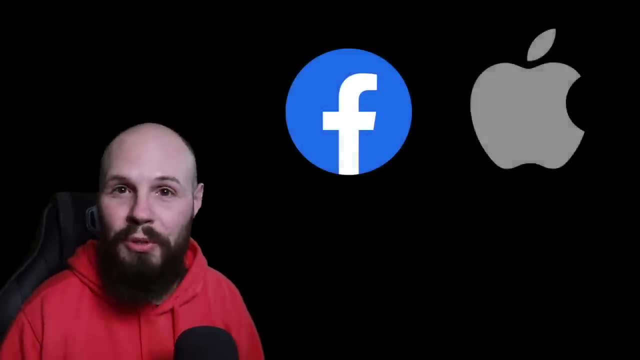 and then I left there to start, and then I left there to start interviewing at some of the major interviewing, at some of the major interviewing, at some of the major companies in Silicon Valley right, the companies in Silicon Valley right, the companies in Silicon Valley right, the Facebook's, the Apple's, the Google's. Facebook's, the Apple's, the Google's. Facebook's, the Apple's, the Google's. naively, I thought I was ready right. naively, I thought I was ready, right. naively, I thought I was ready right. after just a year and a half of. after just a year and a half of. 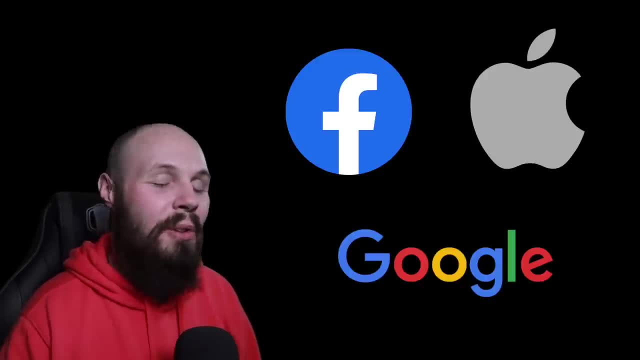 after just a year and a half of basically on the job training, I thought basically on the job training. I thought basically on the job training. I thought I was ready, so I went out and did all I was ready. so I went out and did all I was ready. so I went out and did all those interviews. I got my butt kicked. 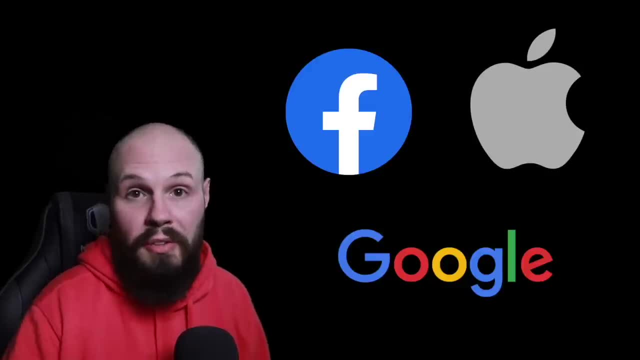 those interviews: I got my butt kicked. those interviews: I got my butt kicked, basically just failed. all those, basically just failed. all those basically just failed. all those interviews: it was a great experience- and interviews: it was a great experience and interviews: it was a great experience and I did get interviews at all these. I did get interviews at all these. I did get interviews at all these companies, but you know when I got to a companies, but you know when I got to a companies, but you know when I got to a final interview or a whiteboarding- final interview or a whiteboarding. 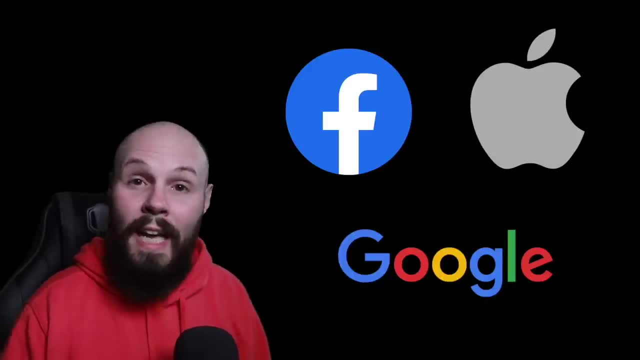 final interview or a whiteboarding session. I got my butt kicked, but it was session. I got my butt kicked, but it was session. I got my butt kicked, but it was a good rude awakening and it actually a good rude awakening and it actually a good rude awakening and it actually led to the creation of my YouTube. 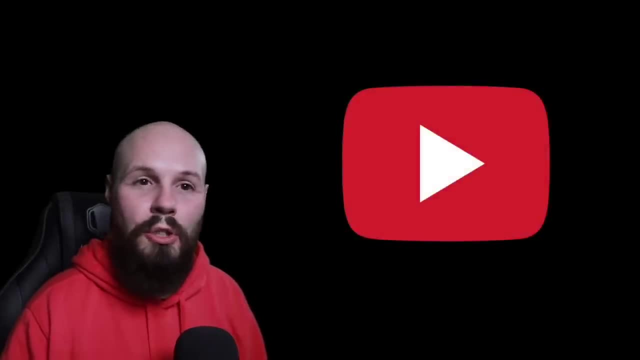 led to the creation of my YouTube, led to the creation of my YouTube channel that many of you are probably channel, that many of you are probably channel, that many of you are probably familiar with, because I wanted to show familiar with, because I wanted to show familiar with, because I wanted to show my knowledge rather than wait on an 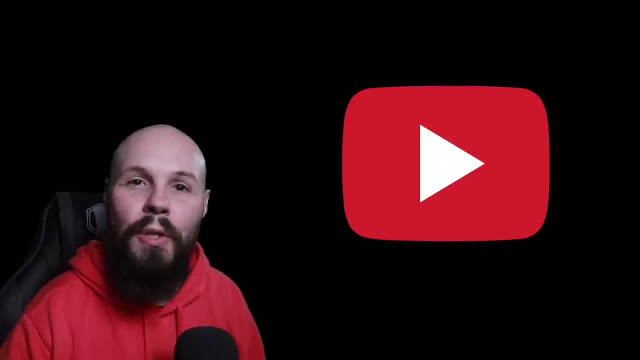 my knowledge rather than wait on an my knowledge rather than wait on an interview. I wanted to just put all my interview. I wanted to just put all my interview. I wanted to just put all my knowledge out there by making videos. knowledge out there by making videos. knowledge out there by making videos, become a well-known name in the space. become a well-known name in the space, become a well-known name in the space, and that was kind of the whole point of and that was kind of the whole point of and that was kind of the whole point of the YouTube channel. but during this time, the YouTube channel, but during this time, 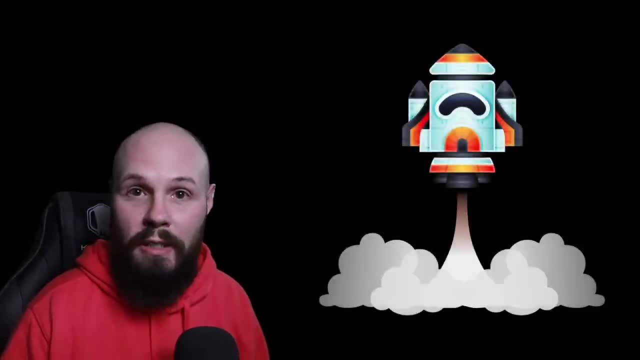 the YouTube channel. but during this time of me getting my butt kicked at, of me getting my butt kicked at, of me getting my butt kicked at interviews, I picked up some contracts, interviews. I picked up some contracts, interviews. I picked up some contracts on the side because I had quit. 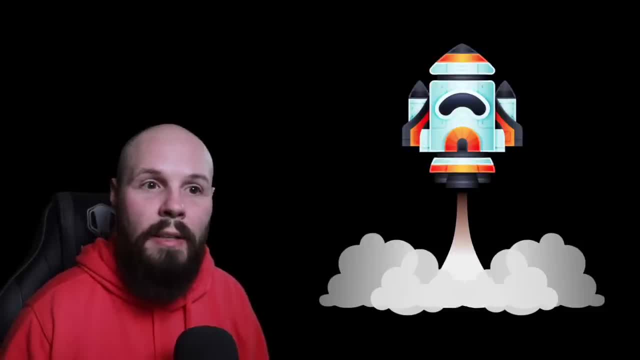 on the side because I had quit on the side. because I had quit breathometer, I wasn't working. I was breathometer. I wasn't working. I was breathometer, I wasn't working. I was focused solely on interviews. and as I'm focused solely on interviews, and as I'm 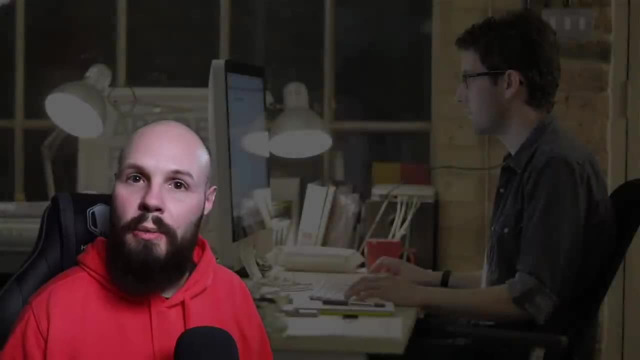 focused solely on interviews and as I'm getting my butt kicked in the interviews- getting my butt kicked in the interviews, getting my butt kicked in the interviews- I started picking up more and more, I started picking up more and more, I started picking up more and more contracts and was like you know what let 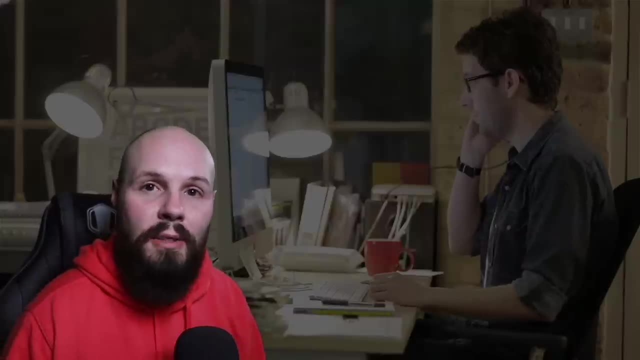 contracts and was like you know what, let contracts. and was like you know what, let me try contracting right. I got enough me try contracting right. I got enough me try contracting right. I got enough to support me. so for the next year and a to support me. so for the next year and a. 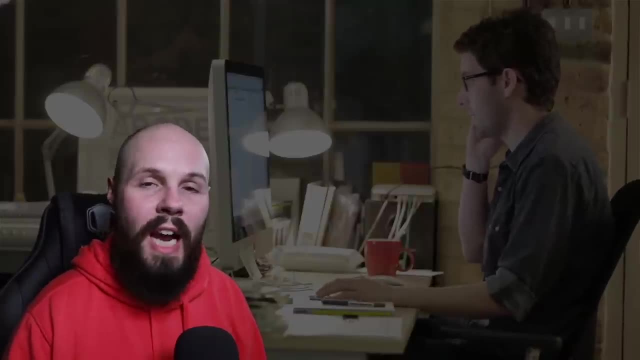 to support me. so for the next year and a half I did independent contracting. half I did independent contracting, half I did independent contracting, which was great. I say that was like the, which was great. I say that was like the, which was great. I say that was like the time where I learned the most, because 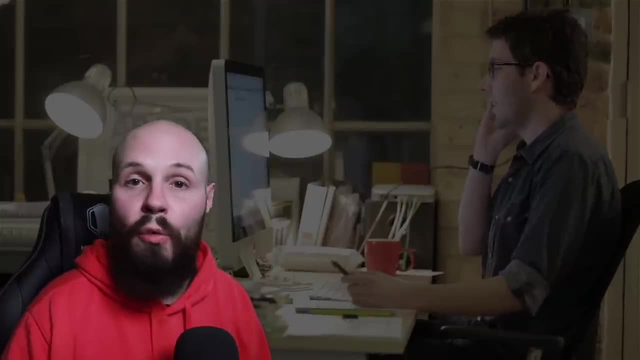 time where I learned the most. because time where I learned the most, because the independent contracting. I bounced the independent contracting, I bounced the independent contracting. I bounced around from project to project like around, from project to project like around, from project to project like every three or four months. so I got a 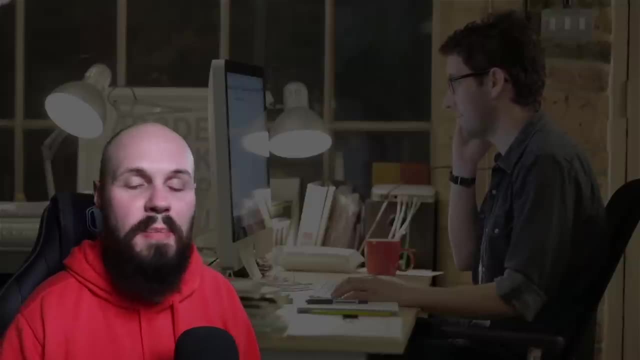 every three or four months. so I got a every three or four months. so I got a lot of experience and a lot of exposure, lot of experience and a lot of exposure, lot of experience and a lot of exposure to different code bases, different types. to different code bases- different types. 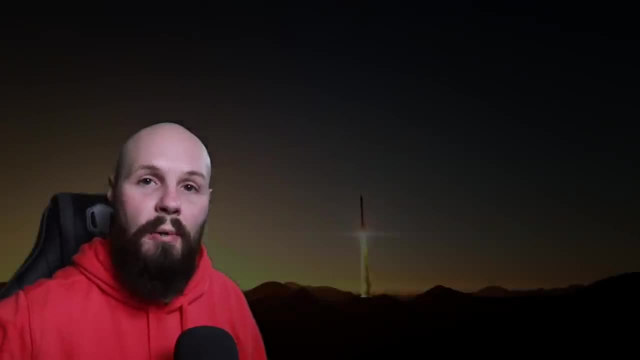 to different code bases, different types of apps, etc. so that's when my learning of apps etc. so that's when my learning of apps, etc. so that's when my learning really skyrocketed, and again at that really skyrocketed, and again at that really skyrocketed, and again at that point I'm already a year and a half into. 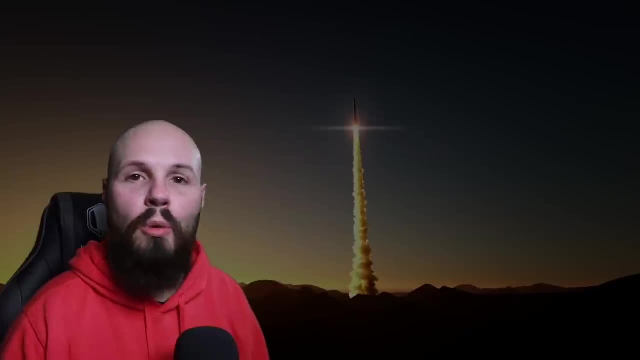 point. I'm already a year and a half into point. I'm already a year and a half into my career before my learning skyrocketed. my career before my learning skyrocketed. my career before my learning skyrocketed. so just keep that in mind, so after. so just keep that in mind, so after. 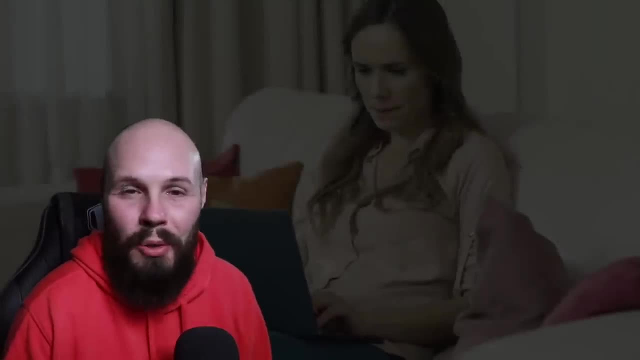 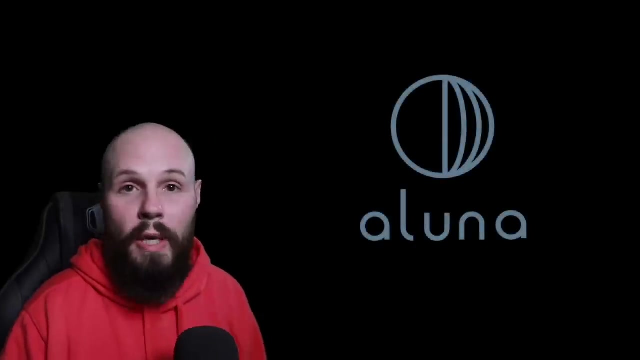 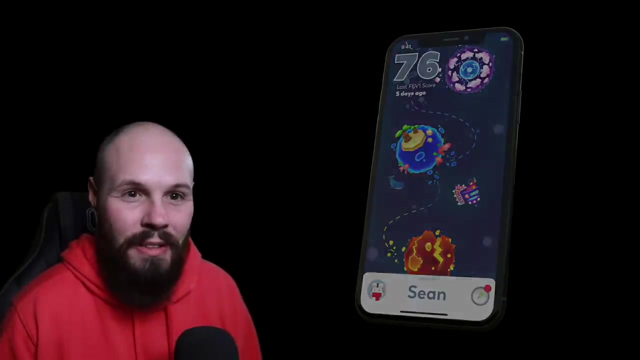 so just keep that in mind. so, after working remotely by myself about a year working remotely by myself, about a year working remotely by myself, about a year and a half, quite frankly, I started and a half, quite frankly, I started and a half, quite frankly, I started working at the Luna back in July of 2019. 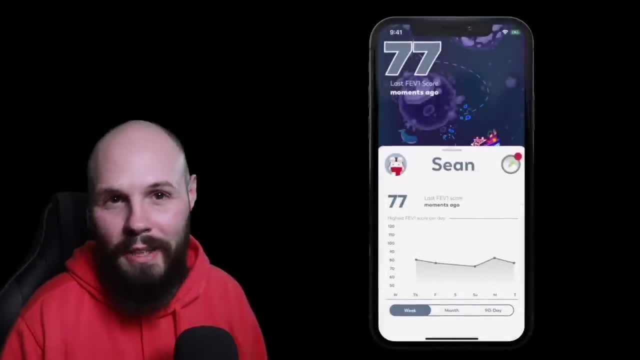 working at the Luna back in July of 2019. working at the Luna back in July of 2019, and I worked there full-time up until- and I worked there full-time up until, and I worked there full-time up until July of 2019. I'm still there to this day. 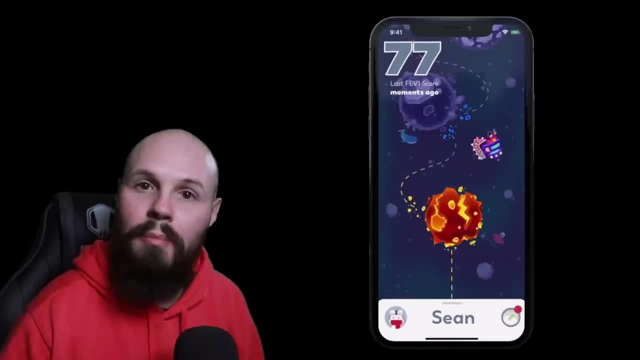 July of 2019. I'm still there to this day, July of 2019. I'm still there to this day in more of a part-time consultancy role, in more of a part-time consultancy role, in more of a part-time consultancy role, because I'm there to like help them make. 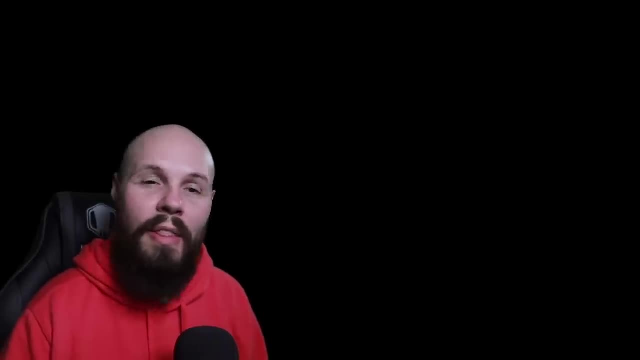 because I'm there to like help them make, because I'm there to like help them make sure the app launches correctly and sure the app launches correctly and sure the app launches correctly and smoothly. but I'm not there full-time smoothly, but I'm not there full-time. 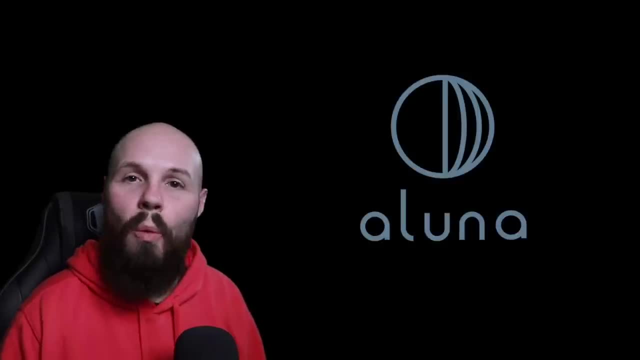 smoothly, but I'm not there full-time anymore now. I left the Luna back in July anymore now. I left the Luna back in July anymore now. I left the Luna back in July of 2019 because I wanted to do one of of 2019, because I wanted to do one of. 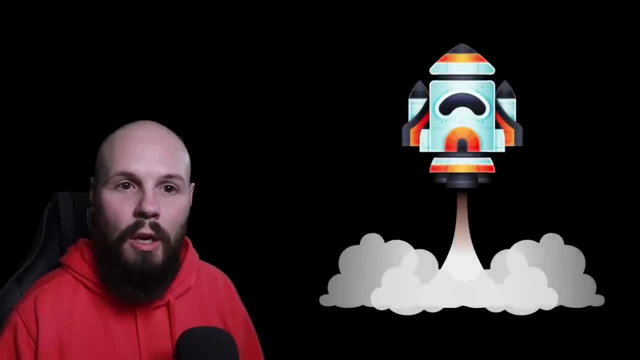 of 2019 because I wanted to do one of two things right. I was kind of at like a two things right. I was kind of at like a two things right. I was kind of at like a crossroads in my career because I'd crossroads in my career because I'd 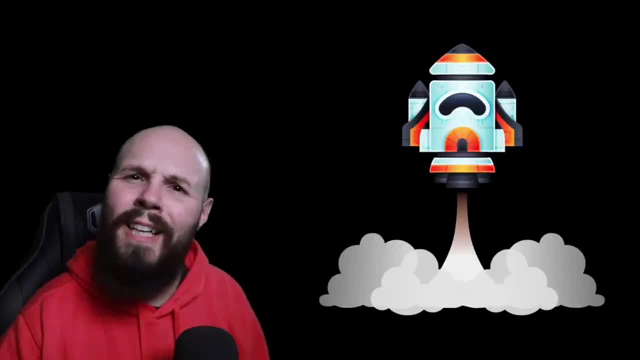 crossroads in my career because I'd spent all my time either independent spent all my time- either independent. spent all my time either independent contracting or at small startups- I contracting- or at small startups- I contracting or at small startups. I never got that experience at a big. 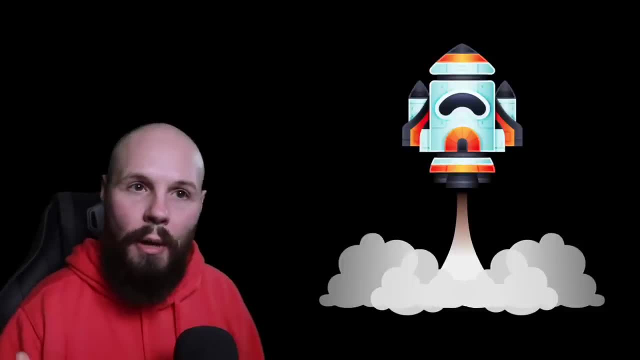 never got that experience at a big, never got that experience at a big company like the Google's, the Facebook's company, like the Google's, the Facebook's company, like the Google's, the Facebook's. so looking back on it, I kind of wanted. so, looking back on it, I kind of wanted. 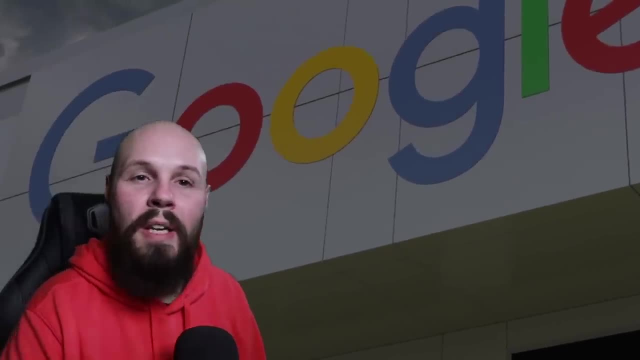 so, looking back on it, I kind of wanted to work there for the wrong reasons. long to work there for the wrong reasons. long to work there for the wrong reasons. long story short. I could either go big story short. I could either go big story short. I could either go big company or pursue this YouTube thing. company or pursue this YouTube thing. company or pursue this YouTube thing full-time, because I, you know, I've been full-time, because I, you know, I've been full-time because I, you know, I've been building this YouTube channel. you know, building this YouTube channel, you know. 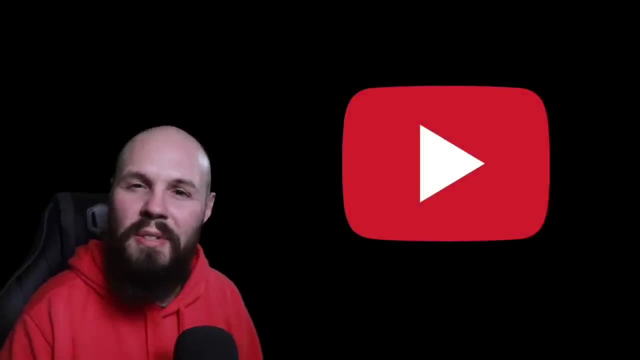 building this YouTube channel. you know, at this time, for like two and a half at this time, for like two and a half at this time, for like two and a half years, it was growing well. I could see years it was growing well. I could see years it was growing well. I could see the business opportunity there. so my 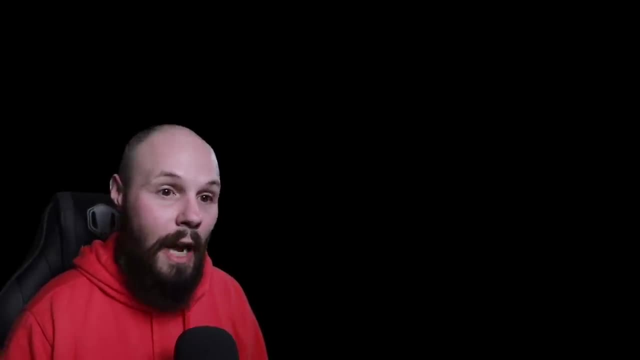 the business opportunity there. so my the business opportunity there. so my choice was: big company: do my own thing. choice was big company: do my own thing. choice was big company: do my own thing. and I was actually in pretty serious and I was actually in pretty serious and I was actually in pretty serious talks with PayPal. I was in the interview. 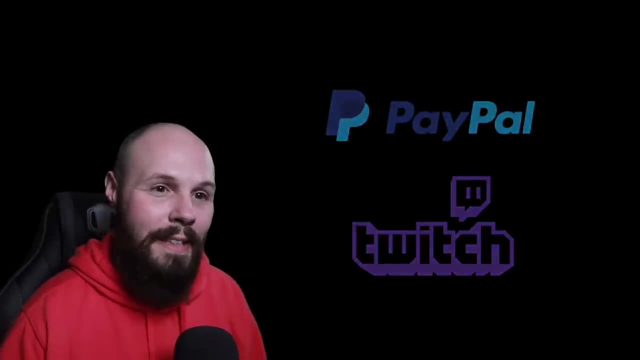 talks with PayPal. I was in the interview talks with PayPal. I was in the interview process with twitch and right in the process with twitch and right in the process with twitch and right in the middle of all that, I decided I'm gonna. middle of all that, I decided I'm gonna. 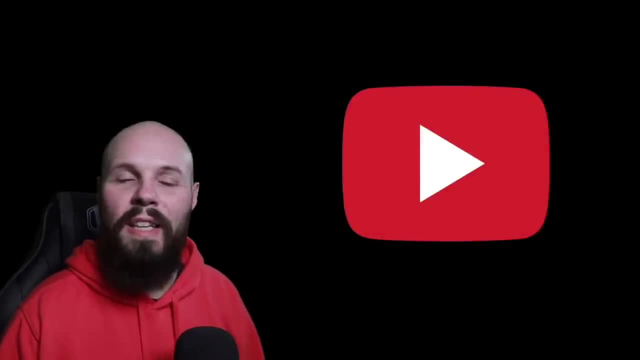 middle of all that, I decided I'm gonna pursue my own thing and do this YouTube, pursue my own thing and do this YouTube, pursue my own thing and do this YouTube thing full-time. so that was back in thing: full-time. so that was back in thing full-time. so that was back in August of 2019. I made the full-time leap. 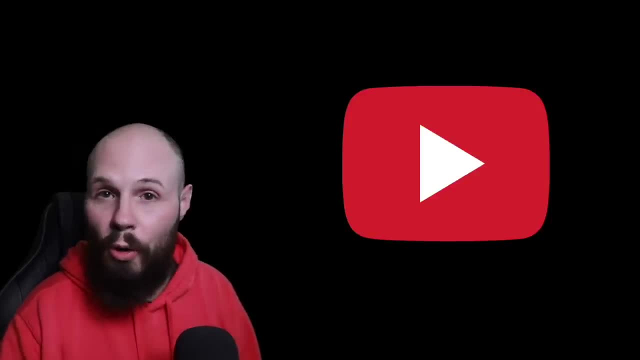 August of 2019, I made the full-time leap. August of 2019, I made the full-time leap. and here we are right: the YouTube. and here we are right, the YouTube. and here we are right, the YouTube channels. going very well, I'm putting out. 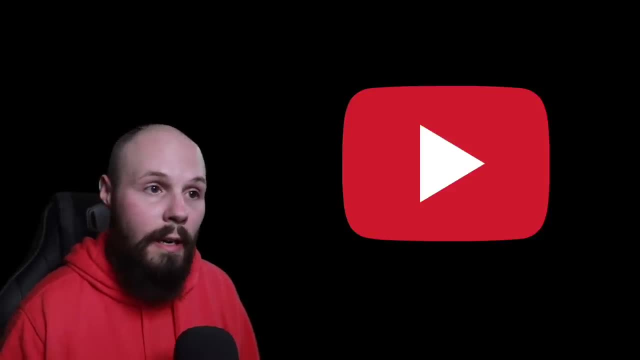 channels going very well. I'm putting out channels going very well. I'm putting out courses for the community, creating all courses for the community. creating all courses for the community, creating all kinds of content for the community. I'm kinds of content for the community. I'm kinds of content for the community. I'm very happy with my decision, right I? 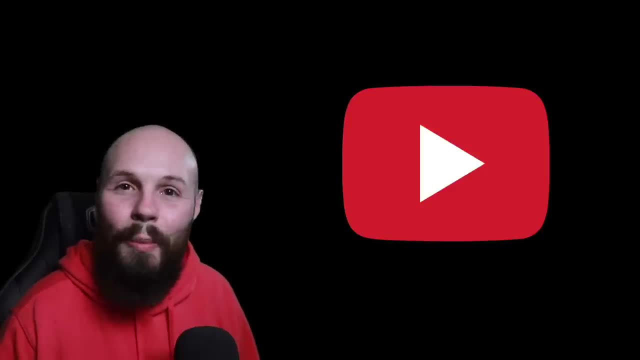 very happy with my decision, right. I very happy with my decision, right. I work for myself. I get to work on fun work for myself. I get to work on fun work for myself. I get to work on fun projects. whatever I think will help my projects, whatever I think will help my. 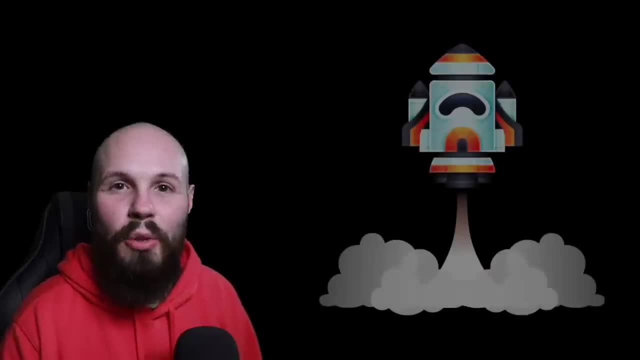 projects, whatever I think will help my YouTube business- it's just a blast. so I YouTube business: it's just a blast. so I YouTube business- it's just a blast. so I was able to take this skill, that I was able to take this skill, that I was able to take this skill, that I learned this iOS development building. 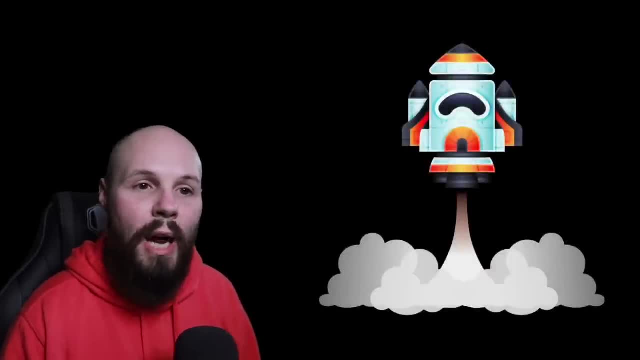 learned this iOS development building. learned this iOS development building products and parlay that over five years products and parlay that over five years products and parlay that over five years into now working for myself again, the into now working for myself again, the into now working for myself again. the biggest benefit of that is I get to work. 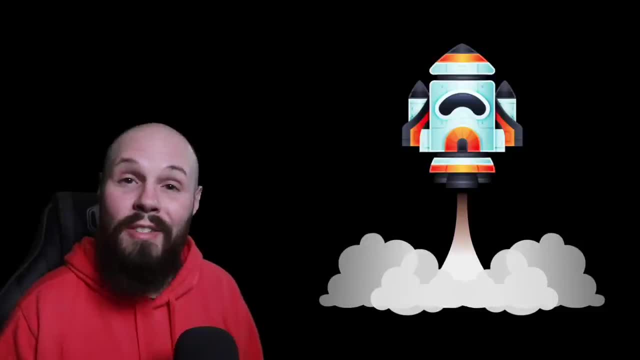 biggest benefit of that is I get to work. biggest benefit of that is I get to work on what I want to work on right. if I on what I want to work on right, if I on what I want to work on right, if I have a cool idea, I work on it and, as of. 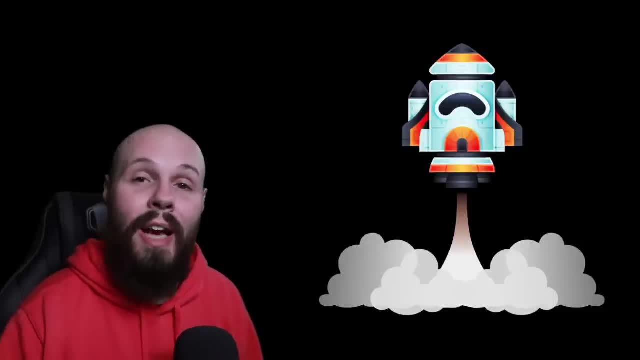 have a cool idea, I work on it. and as of have a cool idea, I work on it. and as of March of 2020, it is already surpassed. my March of 2020: it is already surpassed. my March of 2020: it is already surpassed. my Silicon Valley developer salary and. 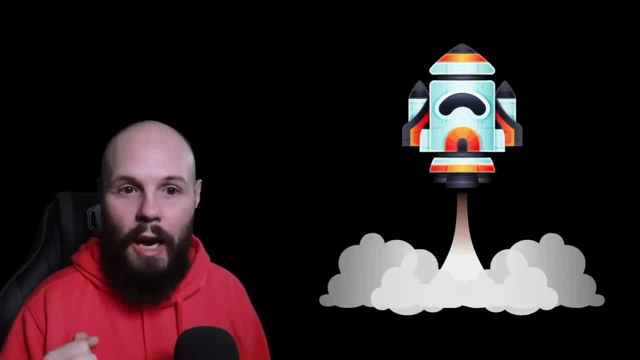 Silicon Valley developer salary and Silicon Valley developer salary and we're still just getting started, so I, we're still just getting started, so I, we're still just getting started. so I don't say that to brag I, I wanted to. don't say that to brag I, I wanted to. 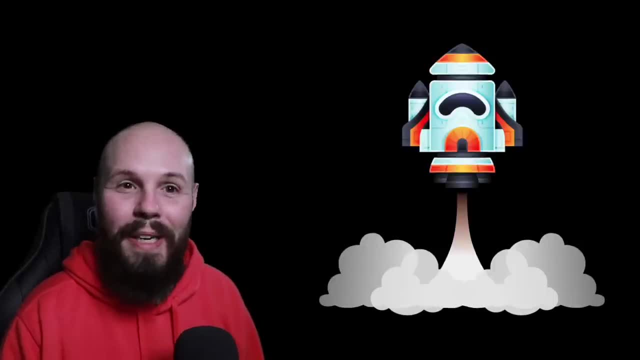 don't say that to brag. I, I wanted to share my story just to show you how share my story, just to show you how share my story, just to show you how great this career is and this skill is great, this career is and this skill is great, this career is and this skill is, and all the flexibility and the things. 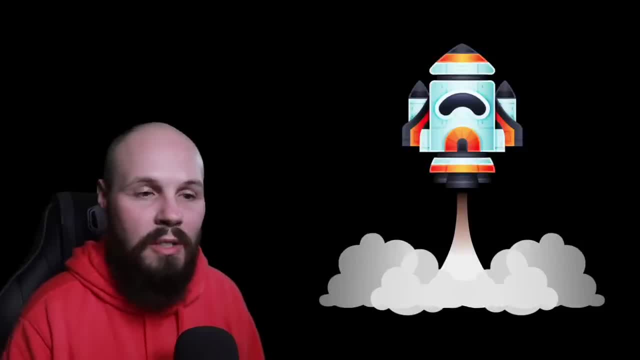 and all the flexibility and the things and all the flexibility and the things you can do, like the multiple career you can do like the multiple career, you can do, like the multiple career, paths you can take with this skill. it's paths you can take with this skill. it's. 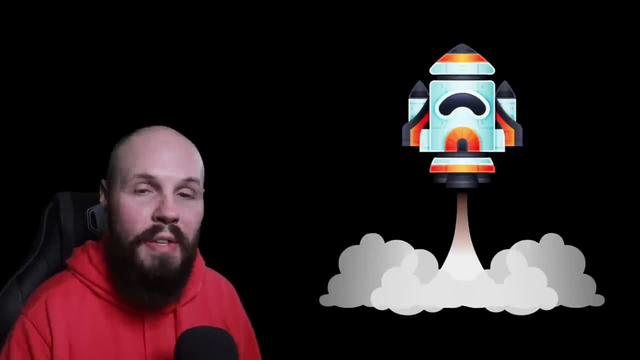 paths you can take with this skill. it's just amazing, in fact. I got a whole. just amazing, in fact, I got a whole. just amazing in fact. I got a whole video later in the course talking about video later in the course talking about video later in the course talking about all the different paths you can take to all the different paths you can take to all the different paths you can take to really you know fit your lifestyle. so really you know fit your lifestyle, so really you know fit your lifestyle. so that's my story and again I wanted to. that's my story and again I wanted to. 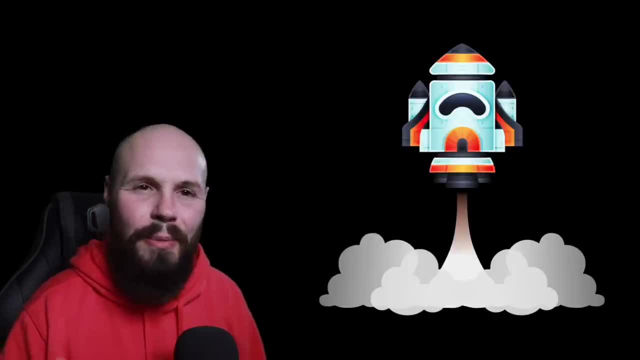 that's my story and again, I wanted to share that to hopefully inspire you, of share that to hopefully inspire you, of share that to hopefully inspire you. of course you're not gonna follow my path course. you're not gonna follow my path course. you're not gonna follow my path directly. you're gonna create your own. 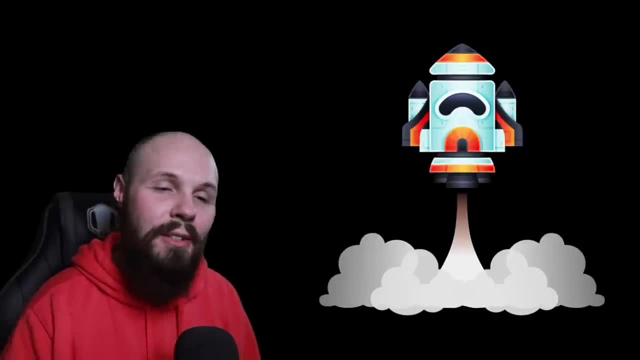 directly. you're gonna create your own. directly. you're gonna create your own path. but the beauty is you have so many path. but the beauty is you have so many path, but the beauty is you have so many options. that path can take you so many options. that path can take you so many. 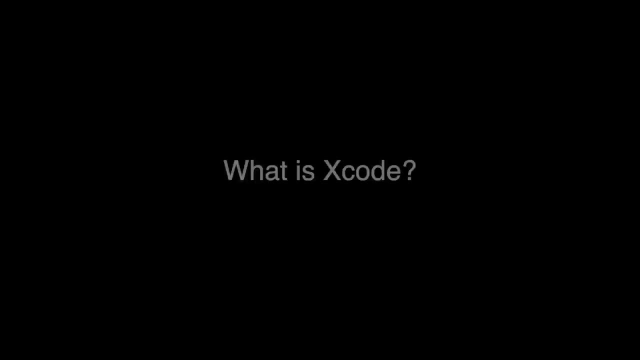 options. that path can take you so many different places, so let's just let's different places. so let's just let's different places. so let's just let's just get on to learning this stuff. just get on to learning this stuff. just get on to learning this stuff, before we can actually start writing. 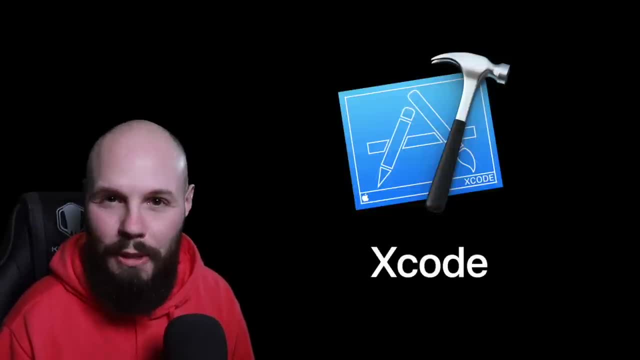 before we can actually start writing, before we can actually start writing Swift code and building apps, we need the Swift code and building apps. we need the Swift code and building apps. we need the tool to do it, and that's Xcode. Xcode is a tool to do it, and that's Xcode. Xcode is a 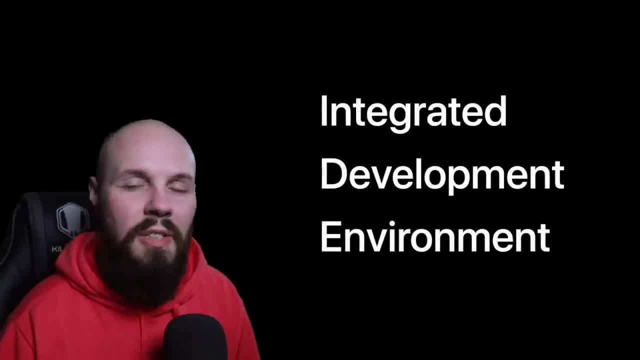 tool to do it, and that's Xcode. Xcode is a IDE or integrated development IDE, or integrated development IDE, or integrated development environment, which basically just means environment, which basically just means environment, which basically just means it's a software program for you to write, it's a software program for you to write. 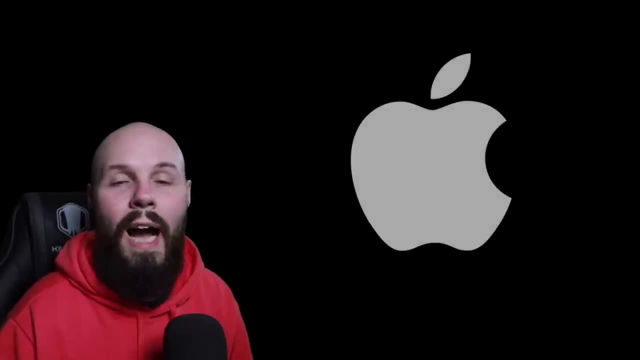 it's a software program for you to write your code, and Xcode is Apple's first your code and Xcode is Apple's first your code and Xcode is Apple's first party IDE that allows you to write code. party IDE that allows you to write code. 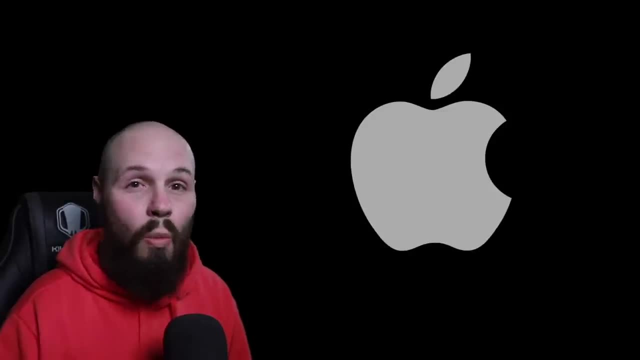 party IDE that allows you to write code for Apple's platforms- right- iOS, Mac OS for Apple's platforms. right, iOS, Mac OS for Apple's platforms. right, iOS, Mac OS, watch OS, you know, etc. and the great watch, you know, etc. and the great watch, you know, etc. and the great thing about this being Apple's first party. 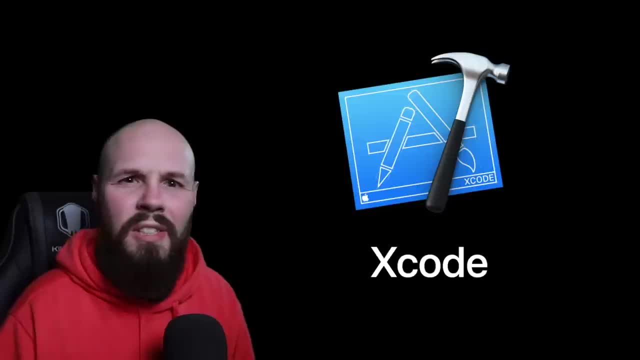 thing about this being Apple's first party thing about this being Apple's first party program is that it's updated program. is that it's updated program, is that it's updated constantly- the typical release cycle, like constantly the typical release cycle, like constantly the typical release cycle, like, for example, we're on Xcode 11, right. 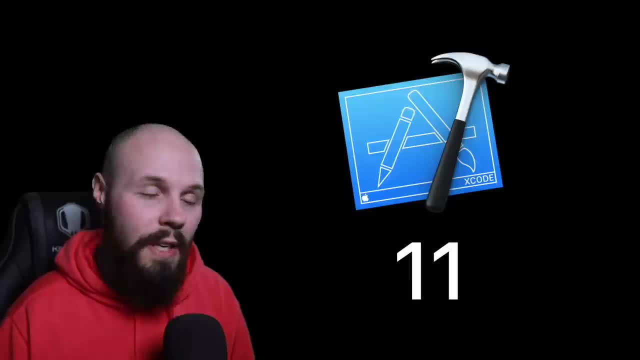 for example, we're on Xcode 11, right. for example, we're on Xcode 11 right now, in March of 2020, but every June you now in March of 2020, but every June you now in March of 2020, but every June, you know the next Xcode gets announced. so 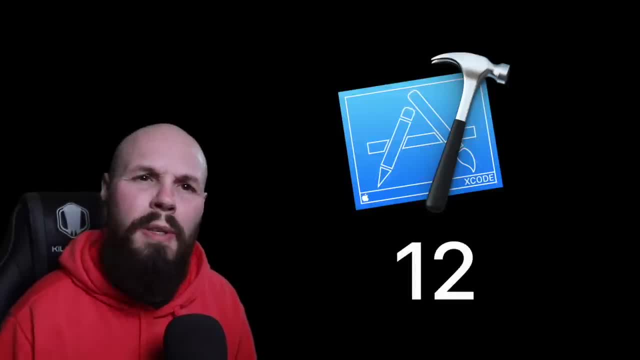 know the next Xcode gets announced. so know the next Xcode gets announced. so Xcode 12 will get announced. that WWDC Xcode 12 will get announced. that WWDC Xcode 12 will get announced that WWDC this year and will be officially. 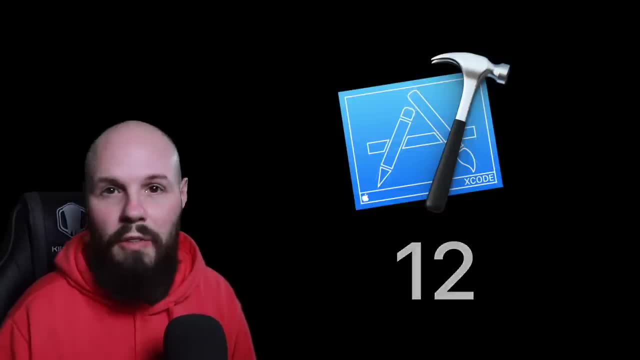 this year and will be officially this year and will be officially released. you know in the fall, but again released. you know in the fall, but again released. you know in the fall, but again it does get updated periodically. it does get updated periodically. it does get updated periodically throughout the year with like Xcode. 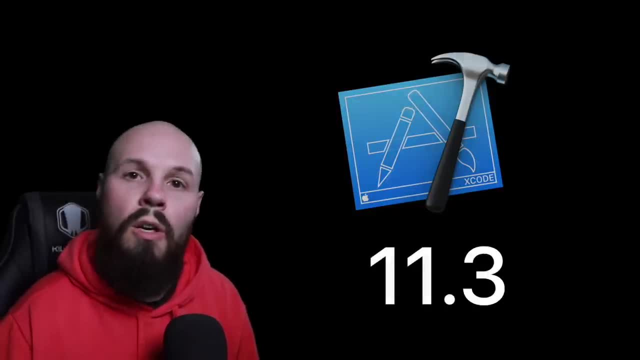 throughout the year with like Xcode throughout the year with like Xcode 11.1, 11.2 and so forth, and here on the 11.1, 11.2 and so forth, and here on the 11.1, 11.2 and so forth, and here on the screen is just what Xcode looks like in. 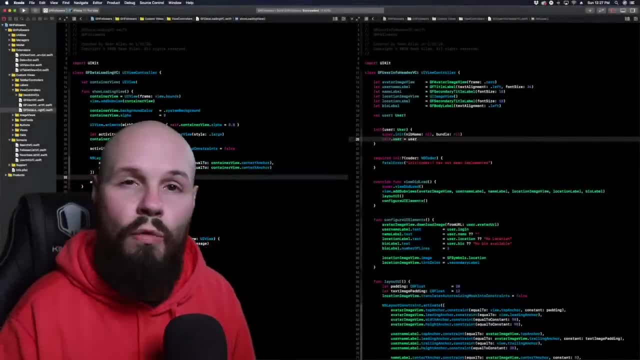 screen is just what Xcode looks like in screen is just what Xcode looks like in a typical project. the project we're a typical project. the project we're a typical project. the project we're looking at right now is the code for my. looking at right now is the code for my. 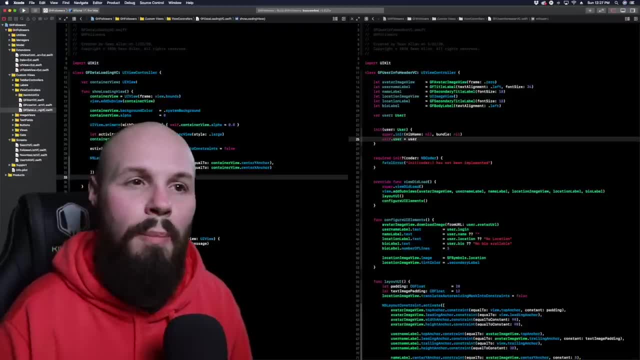 looking at right now is the code for my take-home course and I usually have two take-home course and I usually have two take-home course and I usually have two files of code side-by-side. and if this files of code side-by-side and if this 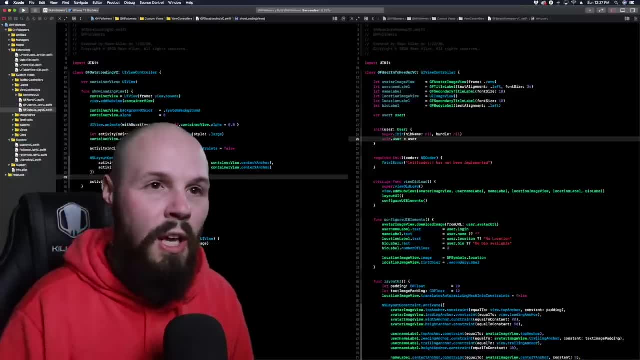 files of code side-by-side. and if this looks a little small, that's because looks a little small. that's because looks a little small, that's because usually when I do a tutorial or a course, usually when I do a tutorial or a course, usually when I do a tutorial or a course, I have my font in my screen resolution. 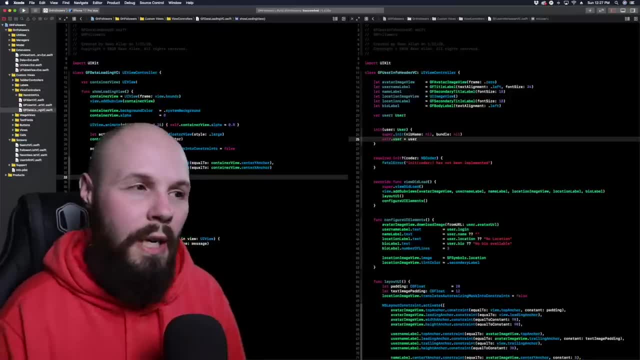 I have my font in my screen resolution. I have my font in my screen resolution blown up so it's easier for you to see blown up, so it's easier for you to see blown up, so it's easier for you to see. but typically when I code it is pretty. 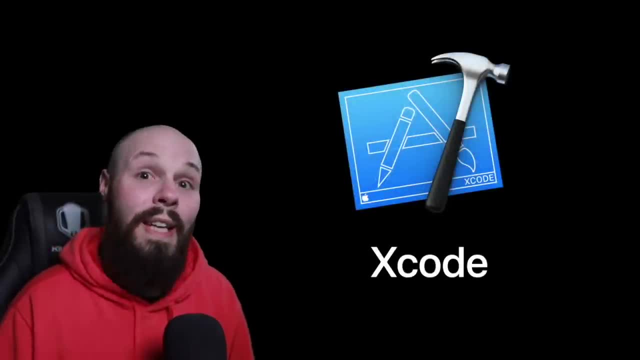 but typically when I code, it is pretty, but typically when I code, it is pretty small like this. so now that you have the small like this, so now that you have the small like this, so now that you have the general idea of what Xcode even is, let's general idea of what Xcode even is. let's general idea of what Xcode even is. let's talk about downloading it first, and talk about downloading it first, and talk about downloading it first and foremost. you're gonna need a Mac, whether foremost, you're gonna need a Mac, whether foremost, you're gonna need a Mac, whether that's a MacBook or an iMac. you're that's a MacBook or an iMac, you're that's a MacBook or an iMac. you're gonna need one of those because Xcode is gonna need one of those because Xcode is. 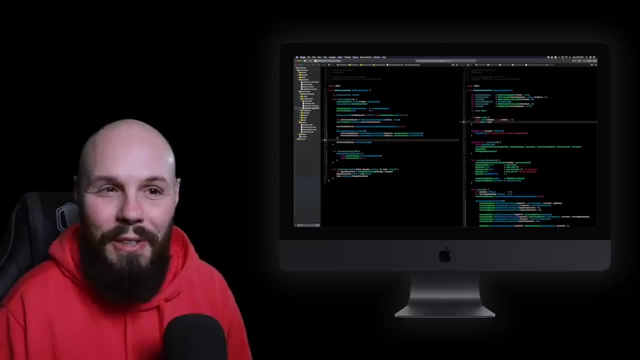 gonna need one of those, because Xcode is meant to run on Mac OS, now, of course. meant to run on Mac OS, now, of course. meant to run on Mac OS, now, of course, with anything with computing. you know, with anything with computing. you know, with anything with computing. you know there are hacky ways to get it to run on. 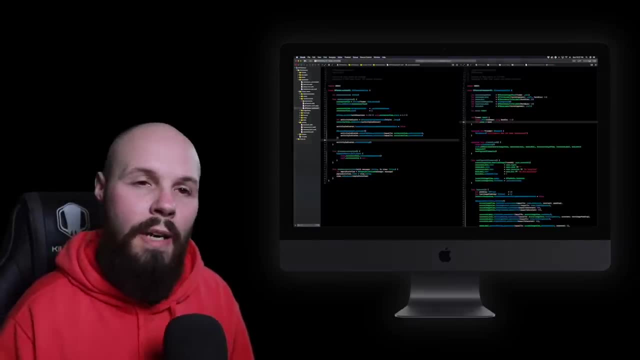 there are hacky ways to get it to run on. there are hacky ways to get it to run on a PC, but that's not recommended to a PC. but that's not recommended to a PC. but that's not recommended to download Xcode on your Mac. go ahead and download Xcode on your Mac. go ahead and download Xcode on your Mac. go ahead and open up the App Store now down in the open up the App Store now down in the open up the App Store now down in the lower left. you know, you should see your. 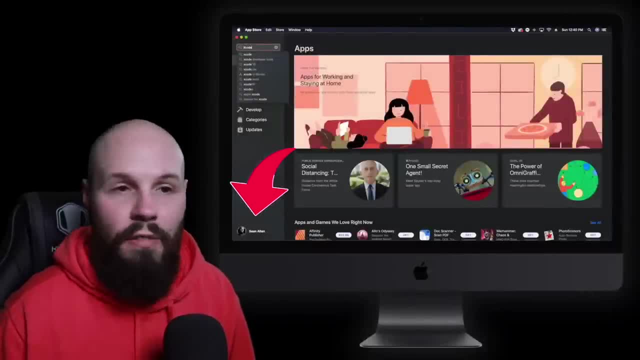 lower left. you know you should see your lower left. you know you should see your name. hopefully, that's if you already name. hopefully, that's if you already name. hopefully, that's if you already have an Apple ID now again, if you have an Apple ID now again, if you already have an iPhone and a Mac, you have an iPhone and a Mac. you have an iPhone and a Mac. you probably have set up your Apple ID, a probably have set up your Apple ID, a probably have set up your Apple ID a long time ago, but just in case you, long time ago. but just in case you. long time ago, but just in case you haven't go ahead and click sign in and haven't go ahead and click sign in and haven't go ahead and click sign in and you have to create your own Apple ID. you have to create your own Apple ID. 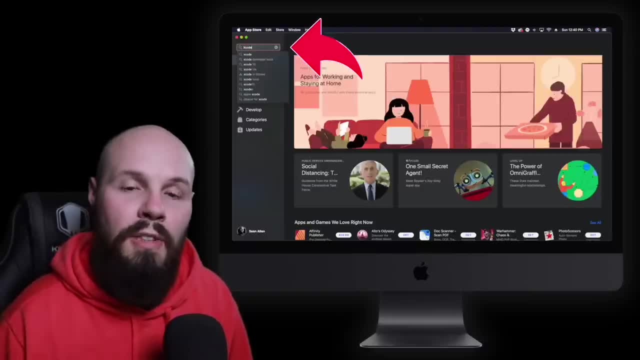 you have to create your own Apple ID there. if you're already signed in, you're there. if you're already signed in, you're there. if you're already signed in, you're good to go in the upper left here type. good to go in the upper left here, type. 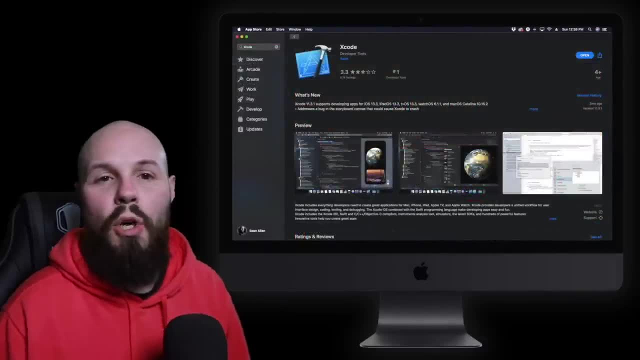 good to go in the upper left here. type in Xcode into the search and you'll see in Xcode into the search and you'll see in Xcode into the search and you'll see it pop up. click on Xcode to open up the. it pop up. click on Xcode to open up the. 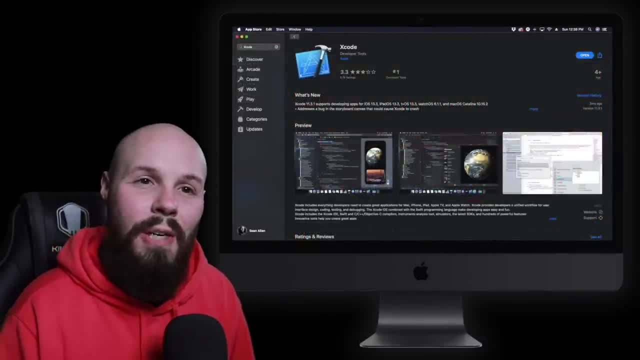 it pop up. click on Xcode to open up the detail page to you know. see a little bit detail page to you know. see a little bit detail page to you know. see a little bit more about it now as you can see down. more about it now as you can see down. 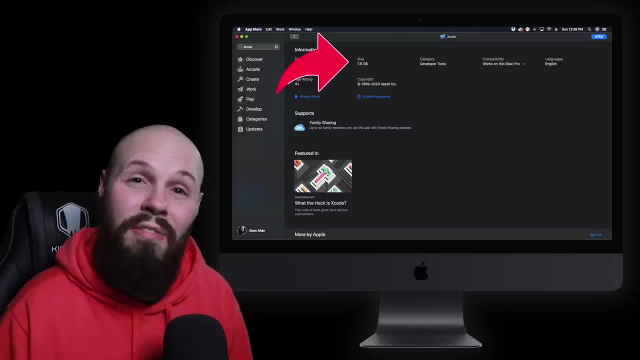 more about it now. as you can see down here, it is 7.8 gigabytes download. so it here. it is 7.8 gigabytes download. so it here. it is 7.8 gigabytes download, so it is a very large file. so make sure you. 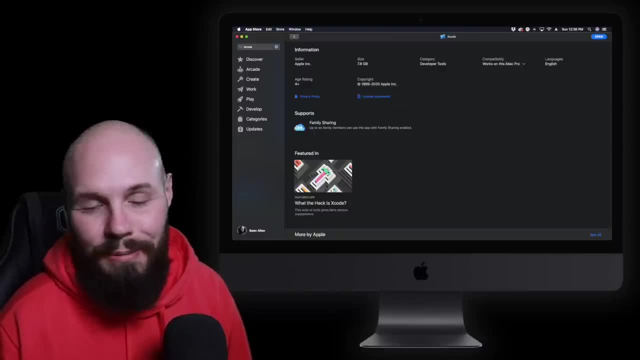 is a very large file, so make sure you is a very large file, so make sure you have enough space for it. and make sure have enough space for it and make sure you got about a half hour to download it. you got about a half hour to download it. 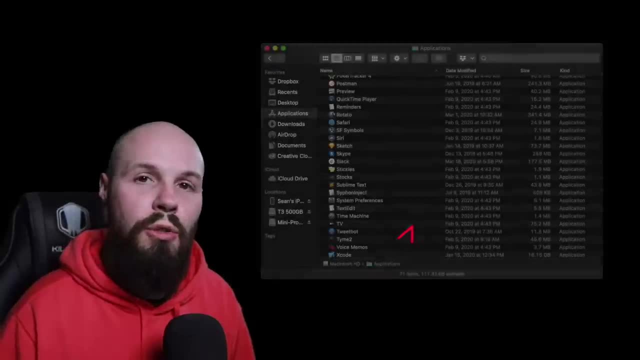 you got about a half hour to download it. you know, depending on your download. you know depending on your download. you know depending on your download speeds after it's finished downloading speeds after it's finished downloading speeds after it's finished downloading. you should see it in your applications. you should see it in your applications. you should see it in your applications folder. go and double click on it to open folder. go and double click on it to open folder. go and double click on it to open it up and you'll see this quick little it up and you'll see this quick little. 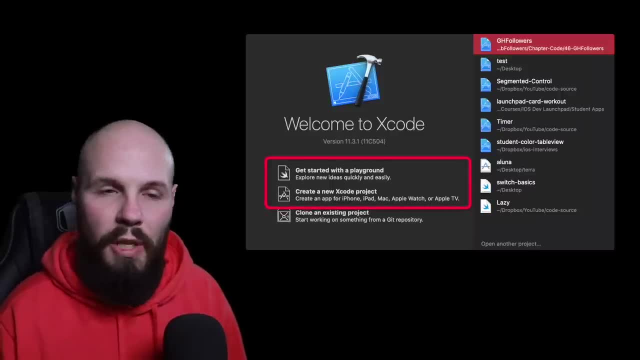 it up and you'll see this quick little menu screen now, as you can see. there's menu screen now, as you can see. there's menu screen now, as you can see, there's two paths we can take. we can create a, two paths we can take. we can create a. 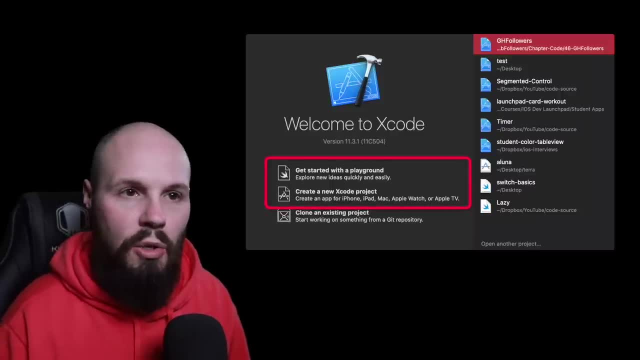 two paths we can take. we can create a new project or create a new playground. new project: or create a new playground, new project or create a new playground. we'll start with a project. so opening up we'll start with a project. so opening up we'll start with a project. so opening up a project is a full-fledged, you know- app. 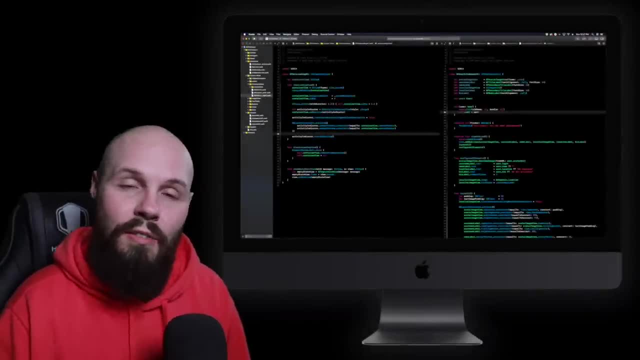 a project is a full-fledged you know app. a project is a full-fledged you know app, whether that's an iphone app, mac os app, whether that's an iphone app, mac os app, whether that's an iphone app, mac os app, watch app, whatever, that's a full-blown. 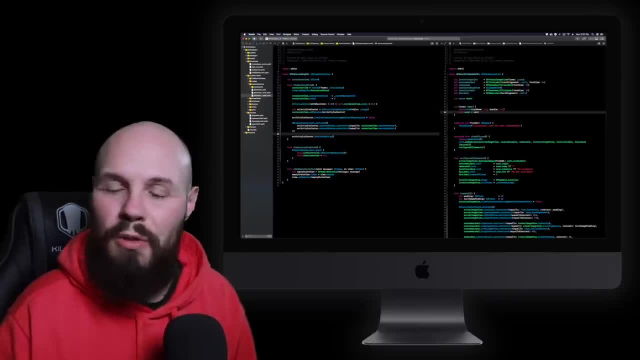 watch app, whatever that's a full-blown watch app, whatever that's a full-blown app app app now, however you may, you know, just want now, however you may, you know, just want now, however you may, you know, just want to play around in some code. to play around in some code. to play around in some code as a matter of fact. that's what we're as a matter of fact. that's what we're as a matter of fact. that's what we're going to do in much of the first half of. 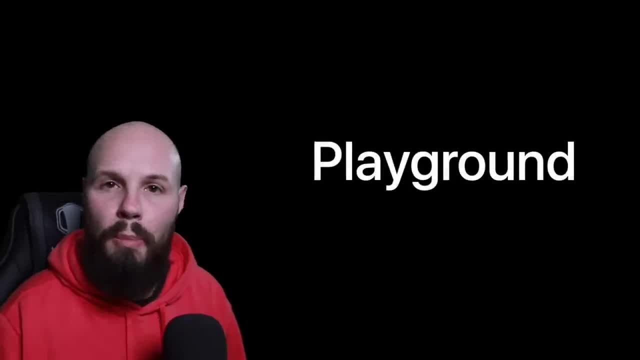 going to do in much of the first half of going to do in much of the first half of this course, when i'm just explaining the this course, when i'm just explaining the this course, when i'm just explaining the basics, that's where you would open up a basics. that's where you would open up a basics. that's where you would open up a playground. you know playground's aptly- playground. you know playground's aptly- playground. you know playground's aptly name: right, it's for you to just go in name. right, it's for you to just go in. 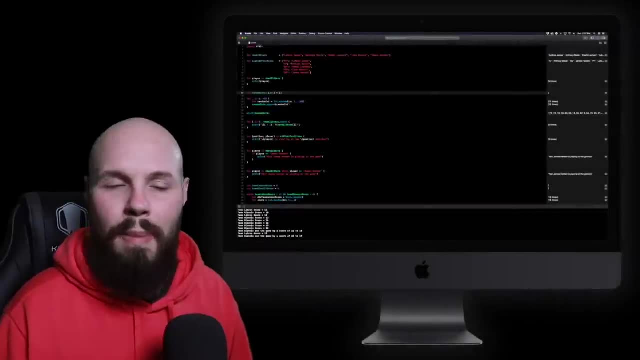 name. right, it's for you to just go in there, play around for a little bit. there, play around for a little bit, there, play around for a little bit. um think of it as kind of like a scratch. um think of it as kind of like a scratch. 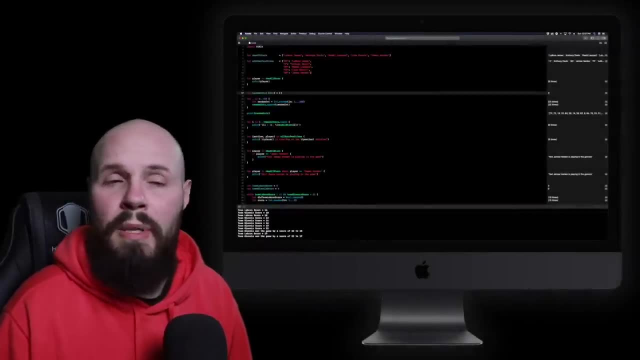 um, think of it as kind of like a scratch pad for your code. if you just want to pad for your code, if you just want to pad for your code, if you just want to try something out, try something out, try something out. but it can't go above and beyond that. 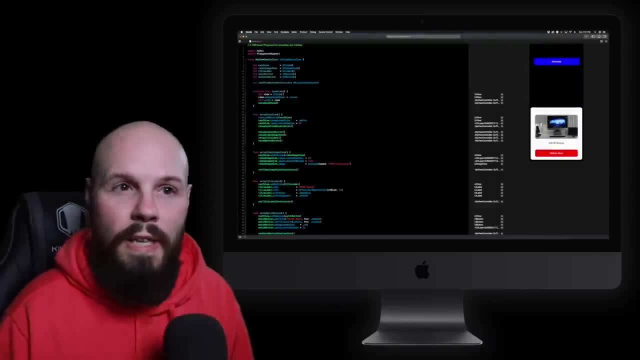 but it can't go above and beyond that. but it can't go above and beyond that. like you can even prototype, like you can even prototype, like you can even prototype ui in a playground, and then, once you've ui in a playground, and then once you've, ui in a playground and then, once you've got the ui tweaked the way you want it, got the ui tweaked the way you want it, got the ui tweaked the way you want it, you can just copy and paste that code. you can just copy and paste that code. 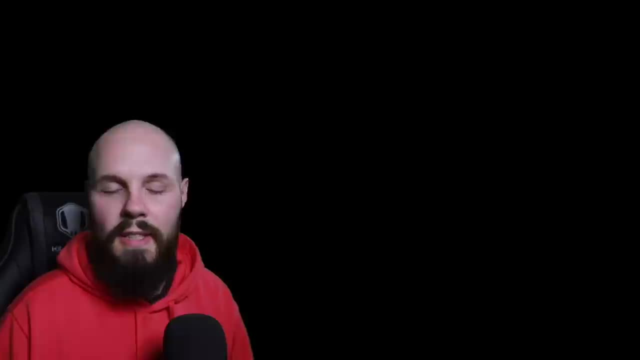 you can just copy and paste that code into your project. so playgrounds are into your project. so playgrounds are into your project. so playgrounds are insanely valuable. so, like i said in this, insanely valuable. so, like i said in this, insanely valuable. so, like i said, in this course we're going to start with. 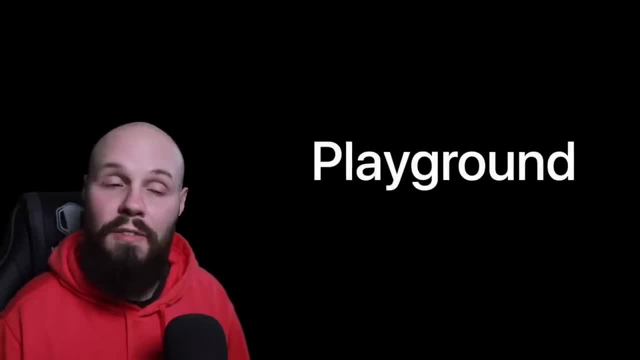 course we're going to start with, course we're going to start with playgrounds, but once we start building playgrounds, but once we start building playgrounds, but once we start building apps, later on we are going to shift apps, later on we are going to shift. 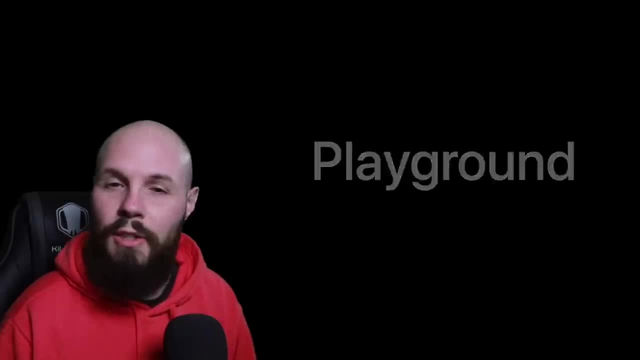 apps. later on we are going to shift into projects where xcode gets a little, into projects where xcode gets a little, into projects where xcode gets a little more complicated, and don't worry when more complicated, and don't worry when more complicated and don't worry when that time comes. i have some separate 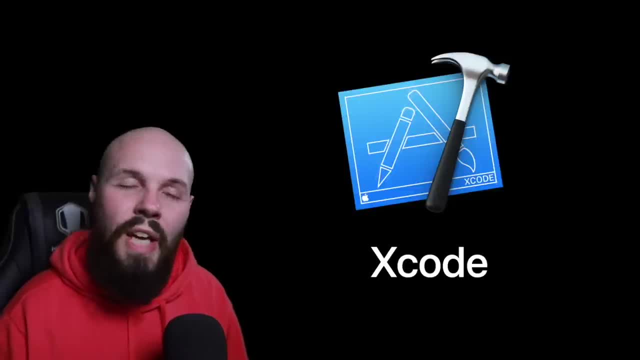 that time comes, i have some separate. that time comes, i have some separate videos. giving a tour of xcode videos. giving a tour of xcode videos. giving a tour of xcode. how to use it: we'll dive into more. how to use it: we'll dive into more. 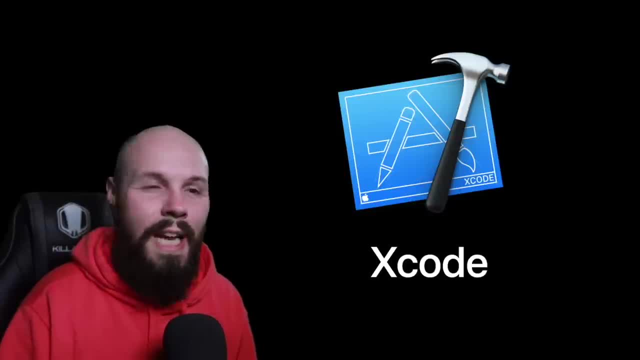 how to use it. we'll dive into more detail on xcode. detail on xcode. detail on xcode then. but i don't want to teach it to you then, but i don't want to teach it to you then, but i don't want to teach it to you now and have you forget it by the time. 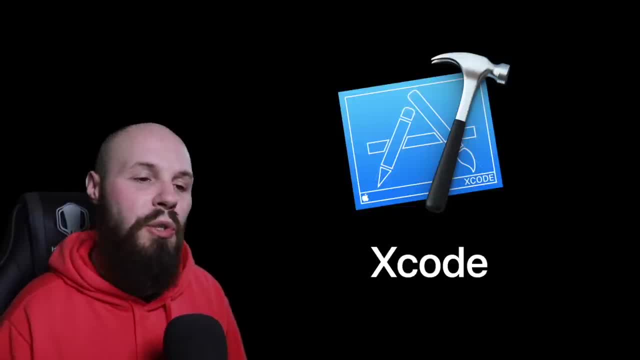 now, and have you forget it by the time now, and have you forget it by the time? we actually use it. so we actually use it, so we actually use it. so we'll push that off till later, but we'll push that off till later, but we'll push that off till later. but there's one thing i want to show you. 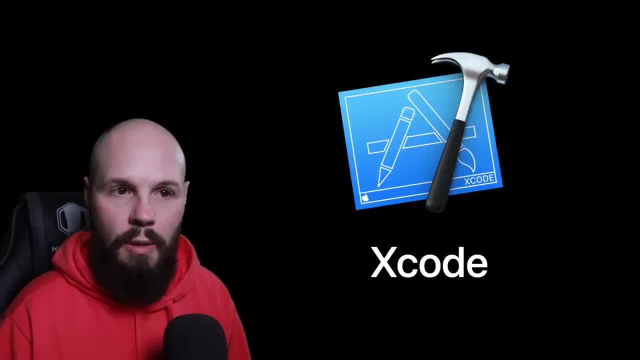 there's one thing i want to show you. there's one thing i want to show you right now because it will affect the right now. because it will affect the right now, because it will affect the playground is your xcode theme. playground is your xcode theme. 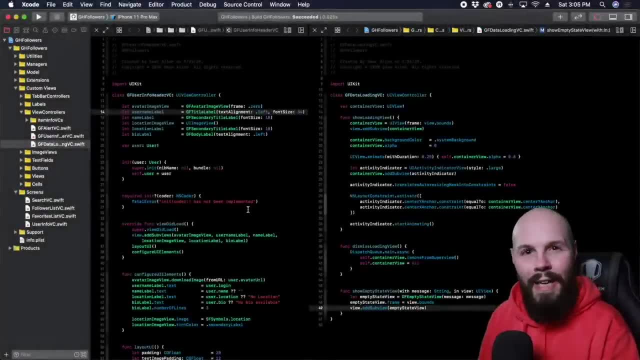 playground is your xcode theme. many of you that just opened up xcode for. many of you that just opened up xcode for many of you that just opened up xcode for the first time you're looking at my, the first time you're looking at my. 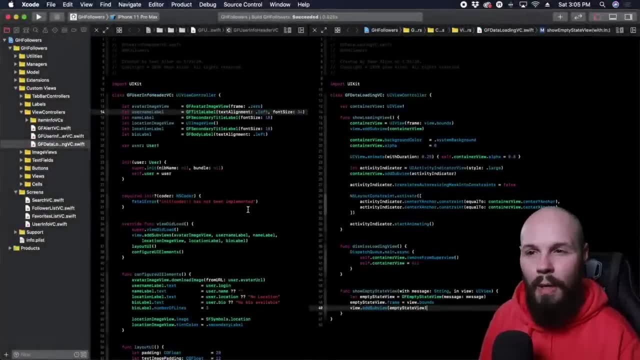 the first time you're looking at my xcode which has a black background, bright xcode which has a black background, bright xcode which has a black background, bright colors. yours may have a white background colors. yours may have a white background colors, yours may have a white background, and you're like: wait a minute, how do i? 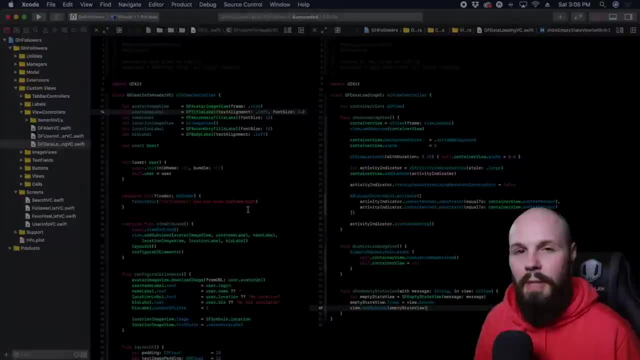 and you're like wait a minute, how do i? and you're like: wait a minute, how do i customize that? how do i get my xcode to customize that? how do i get my xcode to customize that? how do i get my xcode to look like yours? let me show you so back. 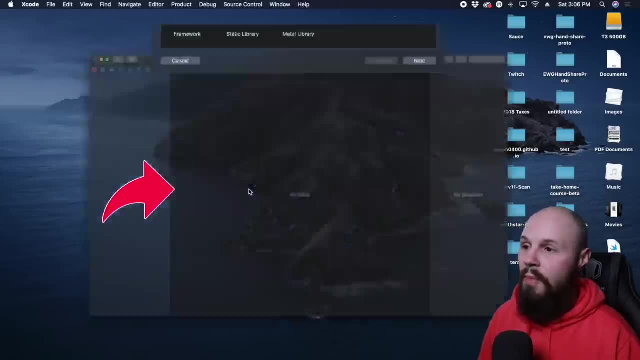 look like yours. let me show you so back. look like yours. let me show you so back in the main xcode menu. go ahead and hit in the main xcode menu. go ahead and hit in the main xcode menu. go ahead and hit create a new xcode project. create a new xcode project. create a new xcode project now. see, you'll get a bunch of options now. see, you'll get a bunch of options now. see, you'll get a bunch of options here: right watch os, tv os, etc. here, right watch os, tv os, etc. here right watch os, tv, os, etc. just open up ios. this is just a test. just open up ios. this is just a test, just open up ios. this is just a test app. we're not really getting into it. you app, we're not really getting into it. you. 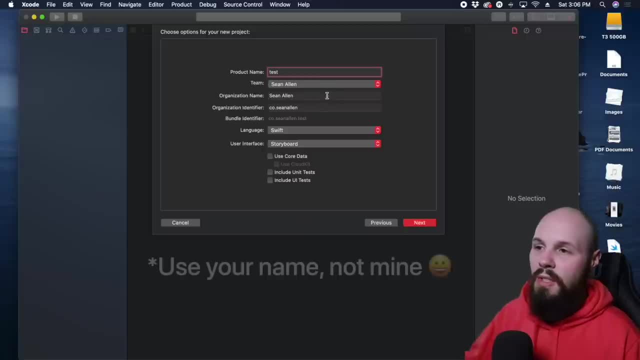 app. we're not really getting into it. you can call it test. can call it test. can call it test. uh, we're going to delete this later. you, uh, we're going to delete this later. you, uh, we're going to delete this later. you can fill out the rest of this based on. 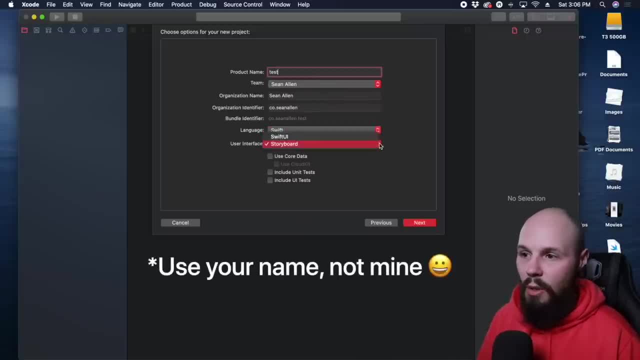 can fill out the rest of this based on. can fill out the rest of this based on my information that i have here. make my information that i have here. make my information that i have here. make sure you have swift selected. sure you have swift selected. sure you have swift selected and storyboard selected, not swift ui. and storyboard selected, not swift ui. and storyboard selected, not swift ui. more on that later again. i'm skimming more on that later again. i'm skimming more on that later again. i'm skimming over this because we're just opening up over this, because we're just opening up. 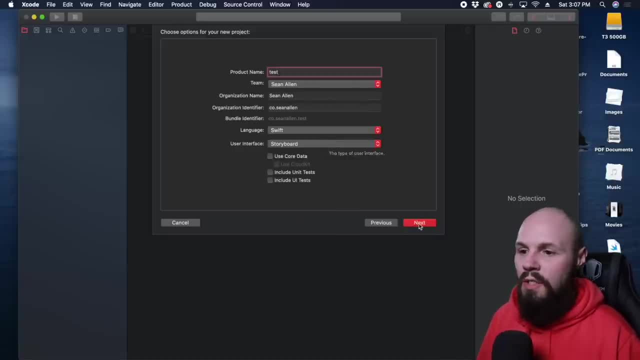 over this, because we're just opening up a quick test project. a quick test project, a quick test project. uh, we will go more in depth later on in. uh, we will go more in depth later on in. uh, we will go more in depth later on in the course. so hit next. 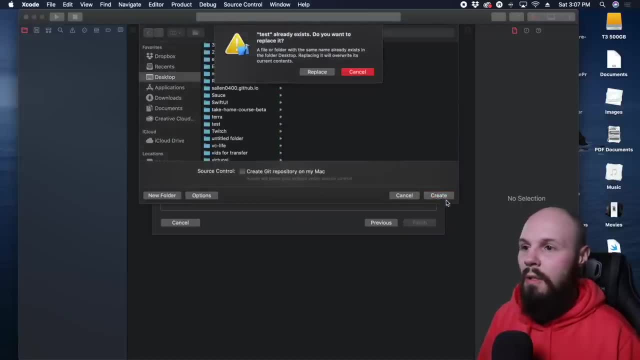 the course, so hit next the course. so hit next uh. and then save it to wherever you like. uh. and then save it to wherever you like, uh. and then save it to wherever you like. i'm going to save it to my desktop. i'm going to save it to my desktop. i'm going to save it to my desktop. i will replace it. i already have a test. i will replace it. i already have a test. i will replace it. i already have a test one because i do this a lot. i will replace it. i already have a test one because i do this a lot. 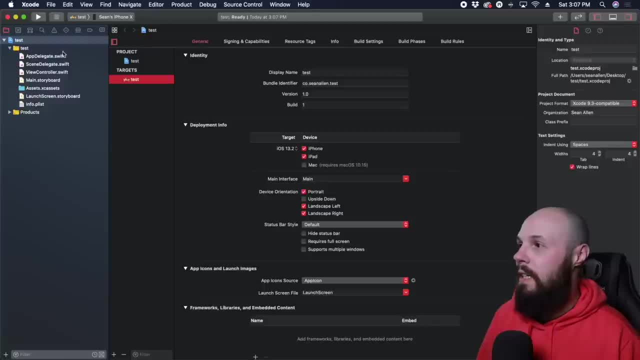 i will replace it. i already have a test one, because i do this a lot. maybe you don't so, maybe you don't so, maybe you don't. so what i want to show you here again is what i want to show you here again is what i want to show you here again is xcode and then preferences. xcode and then preferences: xcode and then preferences. so actually, let me get some code up. so actually, let me get some code up. so actually let me get some code up here. let me go to view controller to get here. let me go to view controller to get. 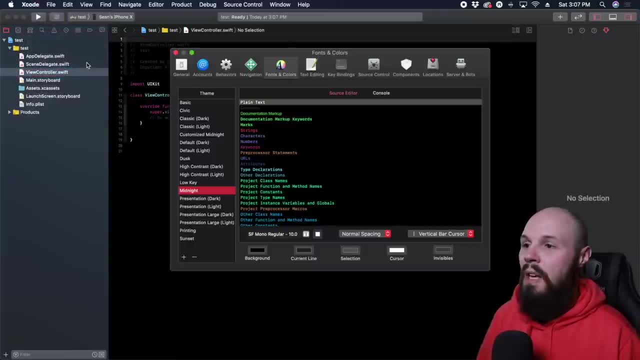 here. let me go to view controller to get some code on the screen and then xcode some code on the screen. and then xcode some code on the screen and then xcode preferences. and you see, here i already preferences. and you see, here i already preferences. and you see, here i already have it selected: fonts and colors, if you. have it selected, fonts and colors. if you have it selected, fonts and colors. if you don't, that's where you want to go and don't that's where you want to go and don't that's where you want to go. and you can see this theme here on the left. 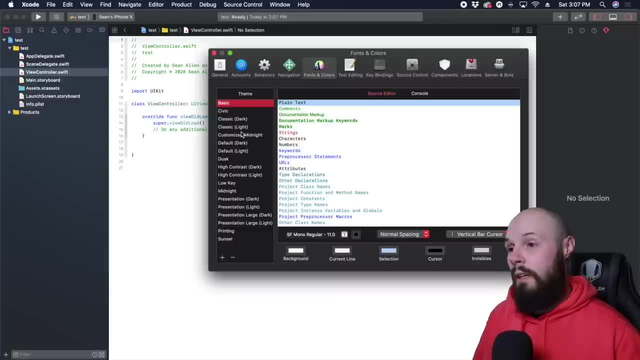 you can see this theme here on the left. you can see this theme here on the left. uh, you probably have it on basic which? uh, you probably have it on basic which? uh, you probably have it on basic- which is a blinding white, is a blinding white. 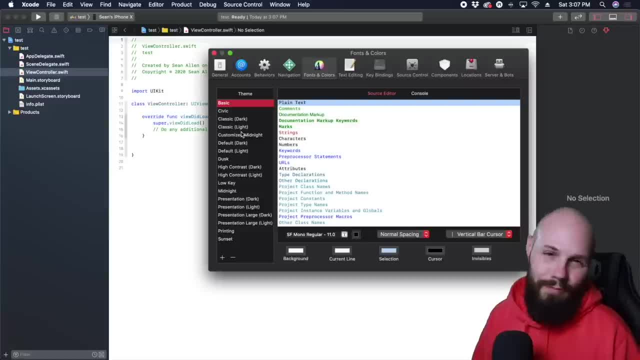 is a blinding white. i only cycle pass. use light mode like i only cycle pass. use light mode like i only cycle pass. use light mode like use dark mode, use dark mode, use dark mode. jokes, of course, but you can see a bunch. jokes, of course, but you can see a bunch. 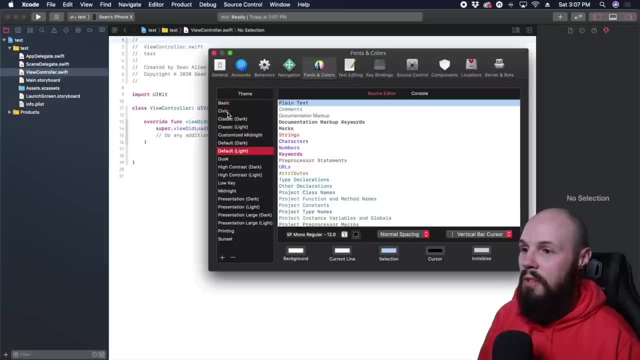 jokes, of course, but you can see a bunch of different themes like civic. i'm just of different themes like civic. i'm just of different themes like civic. i'm just gonna you know page down through these, gonna you know page down through these, gonna you know page down through these, so you can see all the different themes. 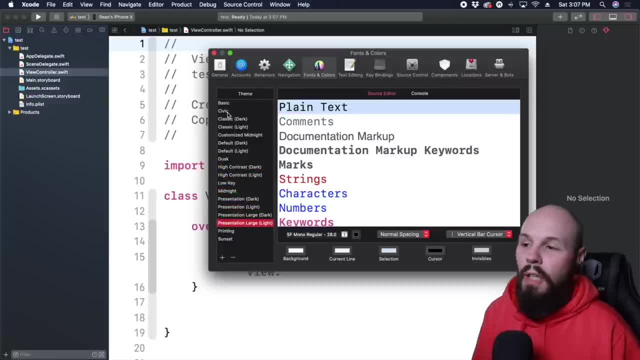 so you can see all the different themes. so you can see all the different themes you can choose. so pick whichever one you, you can choose. so pick whichever one you, you can choose. so pick whichever one you like. again, i was joking, maybe you do like like. again, i was joking, maybe you do like. 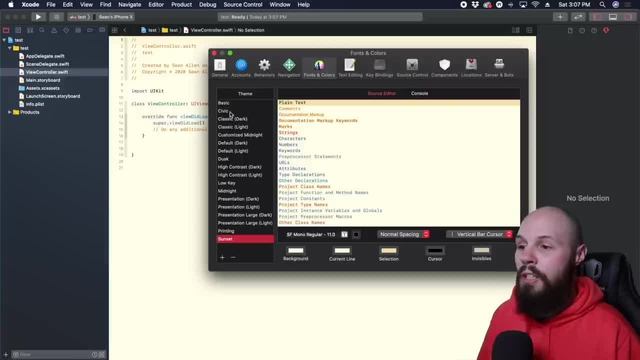 like- again, i was joking, maybe you do like the light background. uh, maybe you like the light background. uh, maybe you like the light background. uh, maybe you like this yellow background, but i choose this yellow background, but i choose this yellow background, but i choose midnight. and then, once you choose your, 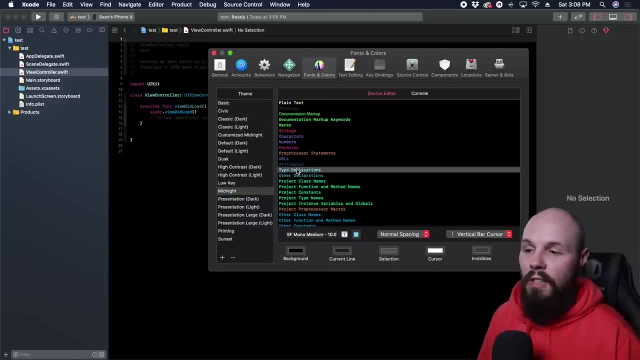 midnight and then once you choose your midnight and then once you choose your theme, you can actually pick each theme. you can actually pick each theme. you can actually pick each individual aspect of that theme and individual aspect of that theme and individual aspect of that theme and customize that even further, down to the 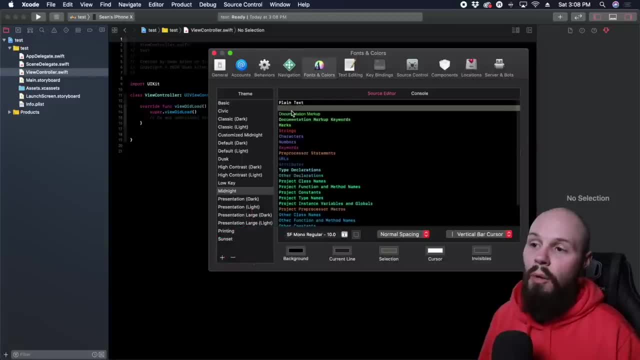 customize that even further down to the. customize that even further down to the font and the color. for example, this font and the color. for example, this font and the color. for example, this comments by default: is this same green comments by default: is this same green comments by default: is this same green that you see here? i like my comments as. that you see here. i like my comments as that. you see here. i like my comments as you can see over here on the left. i like you can see over here on the left, i like you can see over here on the left. i like my comments to kind of fade into the. 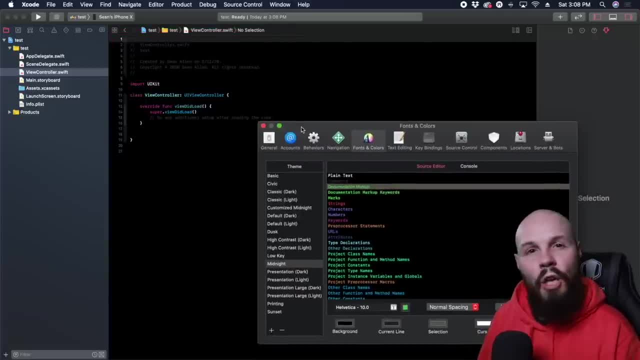 my comments to kind of fade into the, my comments to kind of fade into the background. i don't like them to be you background. i don't like them to be you background. i don't like them to be, you know, overbearing, because i like my code. 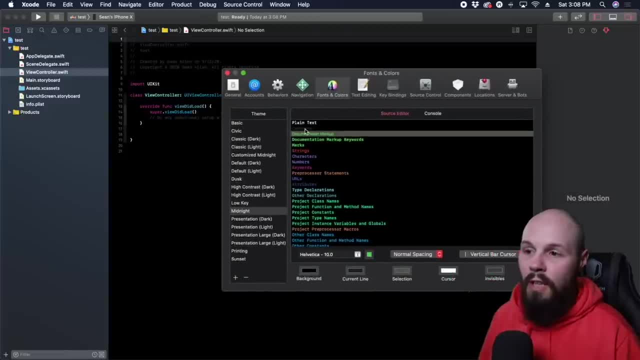 know overbearing, because i like my code know overbearing, because i like my code to actually pop, just my personal to actually pop just my personal, to actually pop, just my personal preference. so what i did was i clicked preference. so what i did was i clicked preference. so what i did was i clicked on comments and then you can click next. 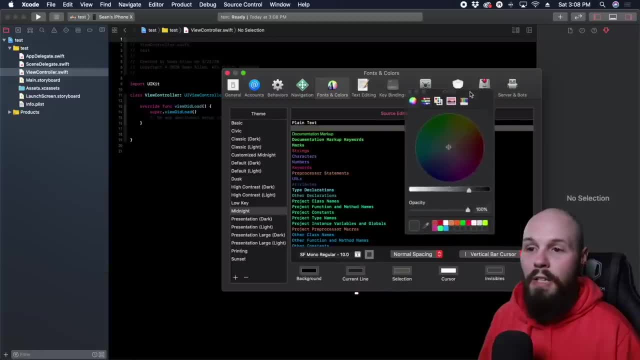 on comments, and then you can click next on comments, and then you can click next to the font here. uh, you can see the to the font here. uh, you can see the to the font here. uh, you can see the color wheel will pop up and then you can. color wheel will pop up and then you can. color wheel will pop up and then you can pick whatever color you want. so keep an pick, whatever color you want. so keep an pick, whatever color you want. so keep an eye on my comments here in the upper. eye on my comments here in the upper. 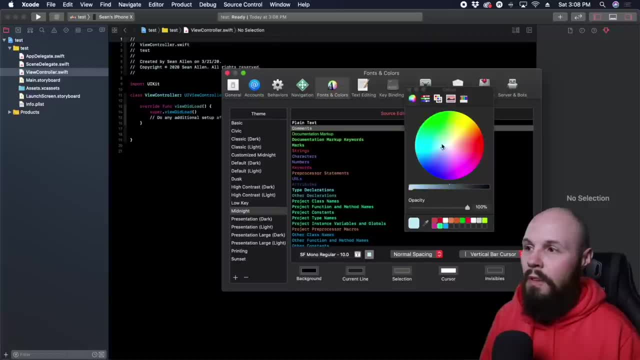 eye on my comments here in the upper left. like, look, i have them blue, we'll left. like, look, i have them blue, we'll left. like, look, i have them blue, we'll have it dark. have it dark, have it dark. right, they can be blue, they can be green. 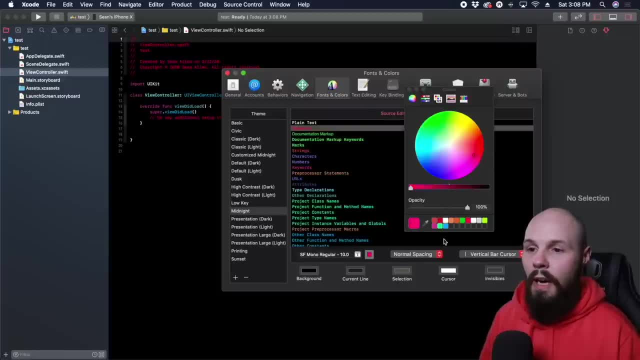 right, they can be blue, they can be green. right, they can be blue, they can be green, yellow red, you can make it whatever you. yellow red, you can make it whatever you yellow red, you can make it whatever you want. again, i uh, i like them to just be. 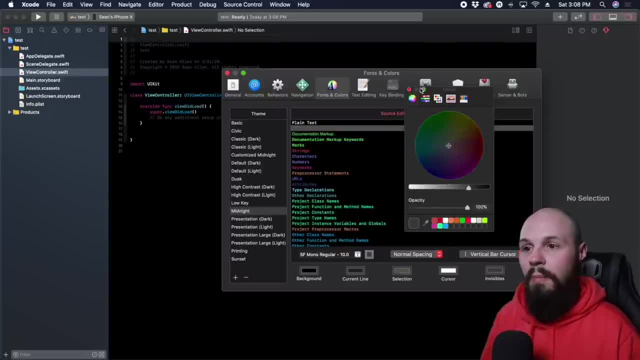 want again. i uh, i like them to just be. want again, i uh, i like them to just be gray so they fade into the background. gray so they fade into the background. gray so they fade into the background. and not be too overbearing. so again if. and not be too overbearing, so again if. and not be too overbearing. so again, if you want to play with your theme to get, you want to play with your theme to get, you want to play with your theme to get it to look right or look like mine. it to look right or look like mine. 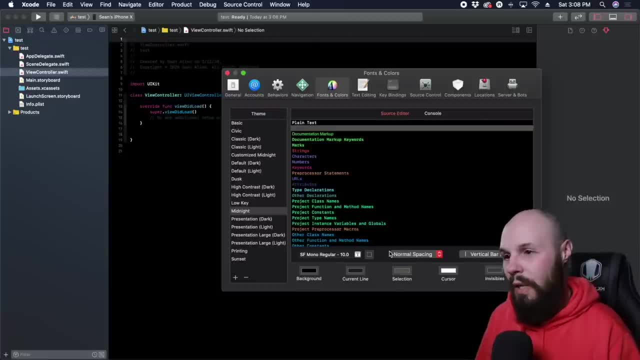 it to look right or look like mine. this is how it's done. have a ball- uh, this is how it's done. have a ball- uh, this is how it's done. have a ball- uh, customize it the way you like. customize it the way you like. customize it the way you like, but this will affect your playgrounds. 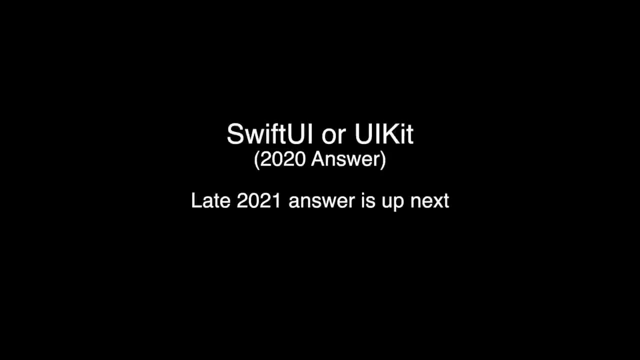 but this will affect your playgrounds. but this will affect your playgrounds. that we'll get into in the next videos. let's take a second to talk about ui kit. let's take a second to talk about ui kit. let's take a second to talk about ui kit versus swift ui. so ui kit is what we've. 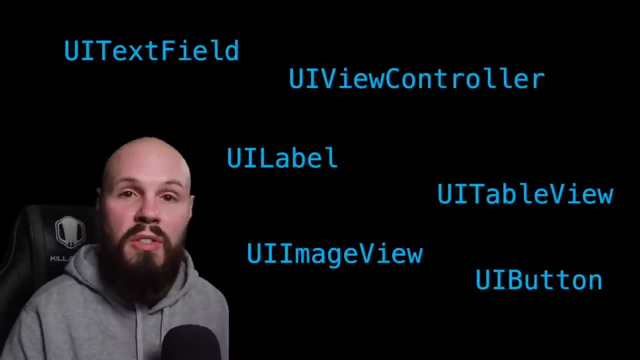 versus swift ui. so ui kit is what we've versus swift ui. so ui kit is what we've used to build our user interfaces in ios. used to build our user interfaces in ios. used to build our user interfaces in ios- development pretty much since it came. development pretty much since it came. 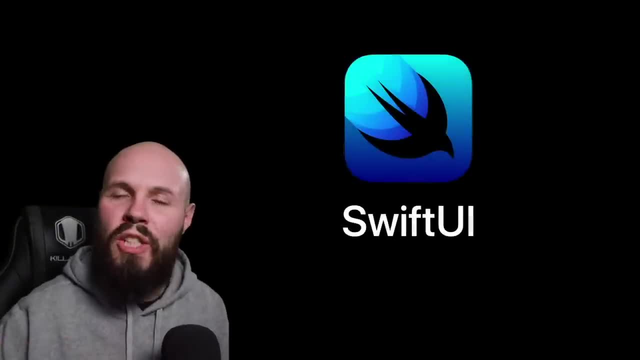 development pretty much since it came out, and swift ui seems to be this new out and swift ui seems to be this new out and swift ui seems to be this new direction that apple's going for all of direction that apple's going for all of direction that apple's going for all of its future development. now we first even 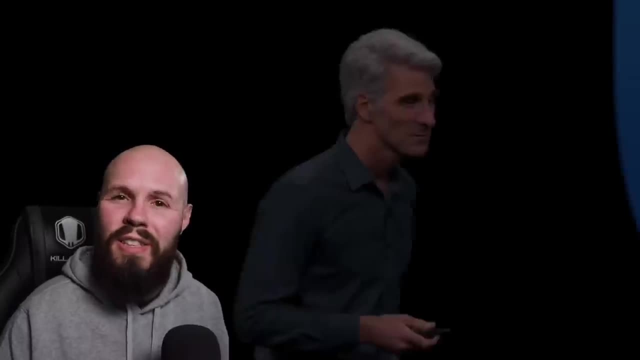 its future development. now we first even its future development. now we first even heard about swift ui in the summer of, heard about swift ui in the summer of, heard about swift ui in the summer of 2019 and it finally just came out of 2019 and it finally just came out of. 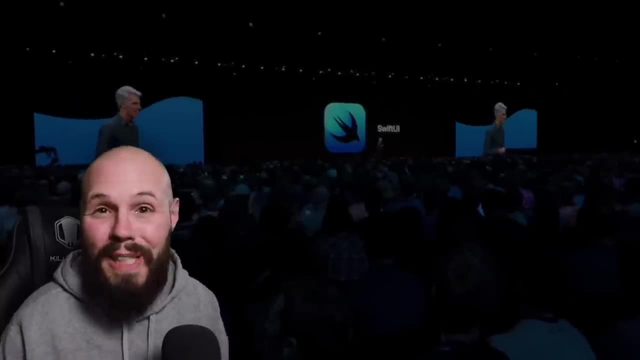 2019 and it finally just came out of beta in fall of 2019, but it is still beta in fall of 2019, but it is still beta in fall of 2019, but it is still extremely early in its development. so extremely early in its development, so. 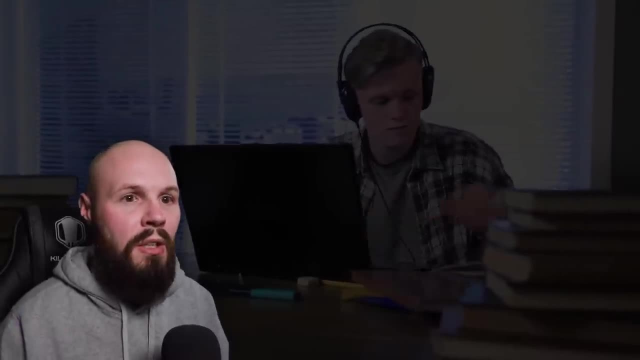 extremely early in its development. so you, as somebody just starting out in ios, you as somebody just starting out in ios, you as somebody just starting out in ios development, you're probably asking what development. you're probably asking what development. you're probably asking what should i learn? should i focus on ui kit? should i learn? should i focus on ui kit? should i learn? should i focus on ui kit or should i focus on swift ui- right? or should i focus on swift ui- right? or should i focus on swift ui- right? because if swift ui is going to be the 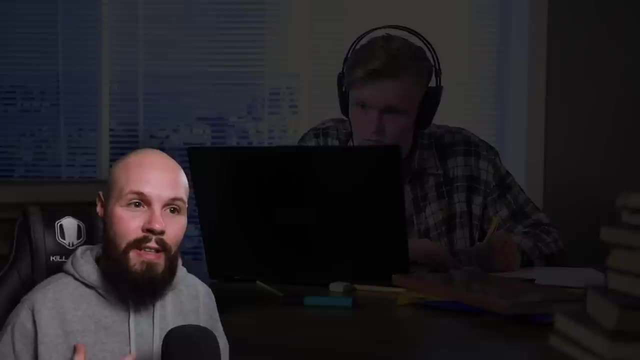 because if swift ui is going to be the, because if swift ui is going to be the future, like i want to focus on where future. like i want to focus on where future. like i want to focus on where apple's going, not where it's been, and 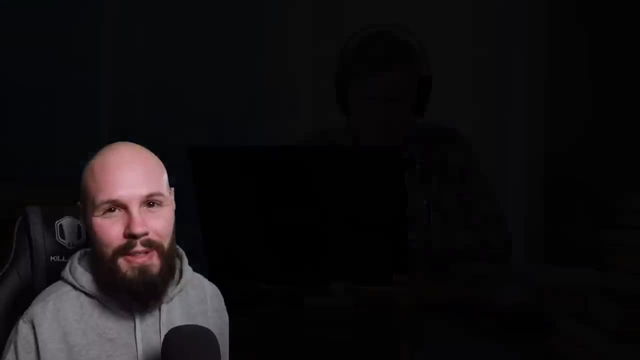 apple's going not where it's been, and apple's going not where it's been, and that makes sense. i get what you're, that makes sense. i get what you're, that makes sense. i get what you're saying, saying, saying. but let's talk about that for a second. 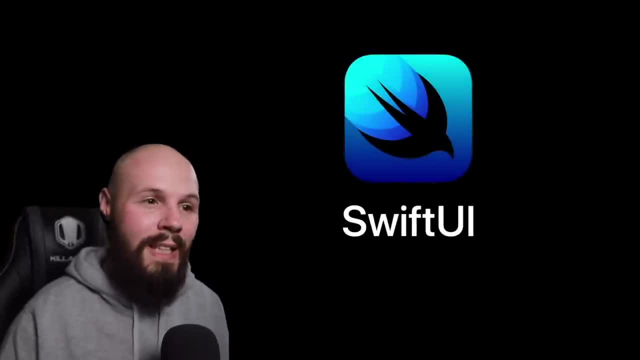 but let's talk about that for a second. but let's talk about that for a second. the bottom line is with swift ui again. the bottom line is with swift ui again. the bottom line is with swift ui again. it's super early in its development. it's. 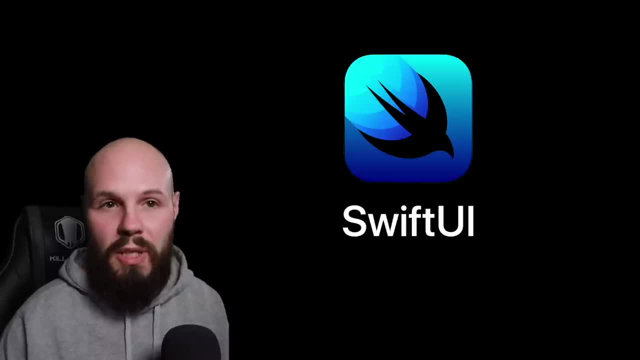 it's super early in its development. it's it's super early in its development. it's not going to be relevant in the job, not going to be relevant in the job, not going to be relevant in the job market, market, market for a couple years. and by relevant, i'm 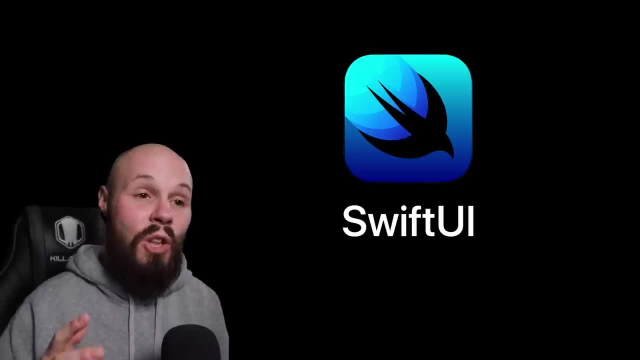 for a couple years, and by relevant i'm for a couple years. and by relevant, i'm not saying there's going to be no swift, not saying there's going to be no swift, not saying there's going to be no swift ui jobs. i'm saying that like a large ui jobs. i'm saying that like a large ui jobs. i'm saying that like a large chunk of jobs will be swift ui and i chunk of jobs will be swift ui and i chunk of jobs will be swift ui and i think that's still, think that's still. 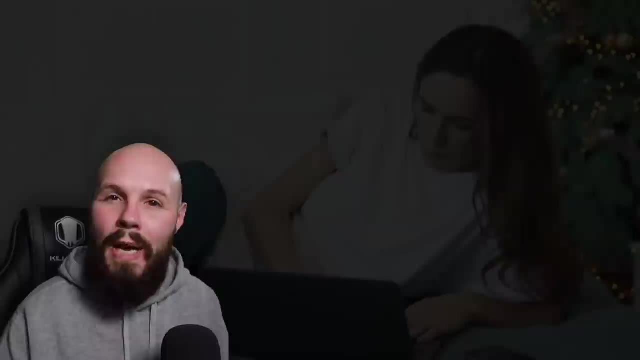 think that's still two, three, four years away, and the two three, four years away and the two three, four years away. and the typical, typical, typical time frame it takes for someone like time frame. it takes for someone like time frame it takes for someone like you who's just learning ios development. you who's just learning ios development, you who's just learning ios development, to get that very first job. to get that very first job, to get that very first job. that can take six months to 18 months to. that can take six months to 18 months to. 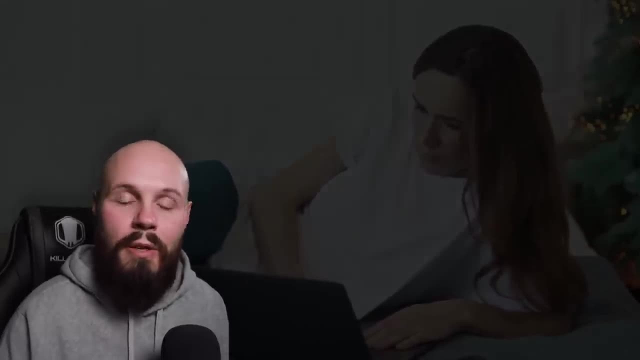 that can take six months to 18 months to even two years. right like that's the even two years. right like that's the even two years. right like that's the typical time frame. so this course is typical time frame. so this course is typical time frame. so this course is coming out in march of 2020, i would say. 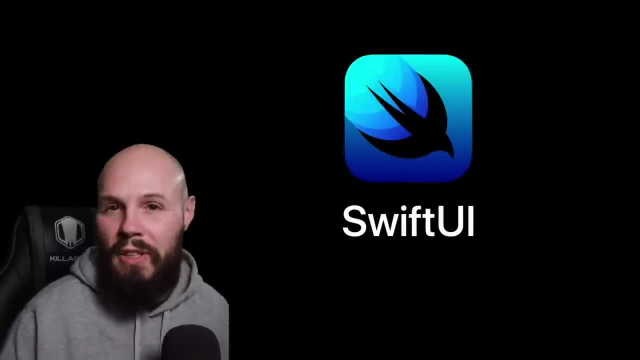 coming out in march of 2020, i would say: coming out in march of 2020, i would say two years from now. swift ui will just be two years from now. swift ui will just be two years from now. swift ui will just be starting to kind of hit its stride. but starting to kind of hit its stride. but starting to kind of hit its stride. but let's think about this for a second. the let's think about this for a second. the let's think about this for a second. the app store has been out for 10 years. app store has been out for 10 years. app store has been out for 10 years and the way we've made apps up till now and the way we've made apps up till now and the way we've made apps up till now is with ui kit. so that is millions of. 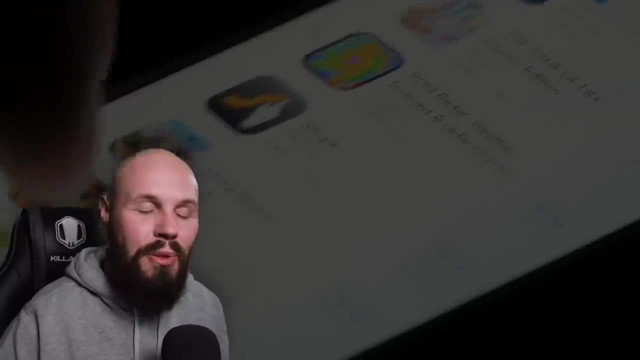 is with ui kit, so that is millions of is with ui kit, so that is millions of ios apps built in ui kit. but even next ios apps built in ui kit, but even next ios apps built in ui kit. but even next year, two, three, four years from now, when 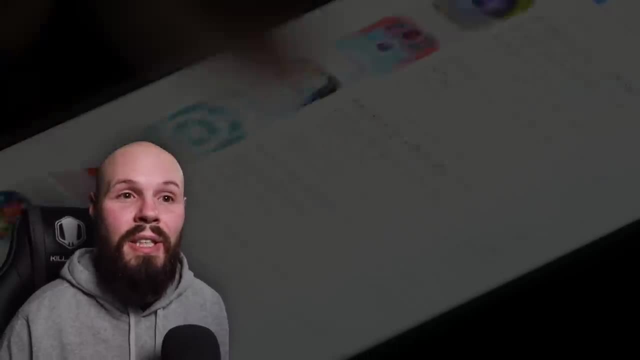 year two, three, four years from now. when year two, three, four years from now, when you're out in the job market- there's, you're out in the job market, there's, you're out in the job market- there's still an extremely high likelihood that still an extremely high likelihood that. 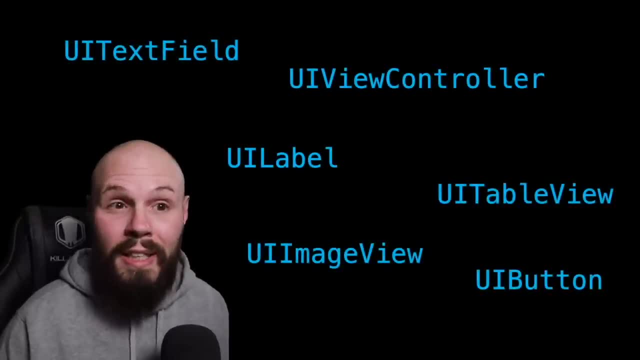 still an extremely high likelihood that the app you get hired for, the app you get hired for, the app you get hired for- will be either all ui kit or still have will be either all ui kit or still have will be either all ui kit or still have a lot of ui kit. so 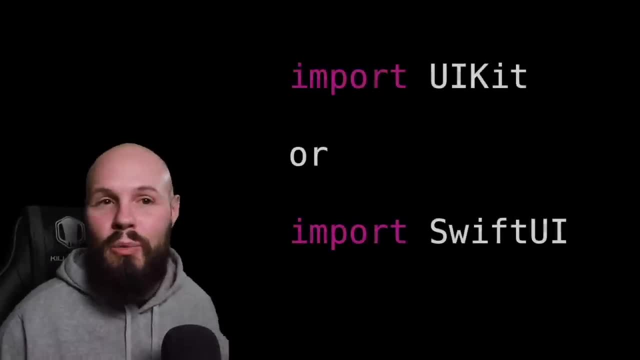 a lot of ui kit, so a lot of ui kit. so the bottom line is you know you're the bottom line, is you know you're the bottom line is you know you're asking yourself which one should i learn? asking yourself, which one should i learn? asking yourself, which one should i learn? ui kit or swift ui? 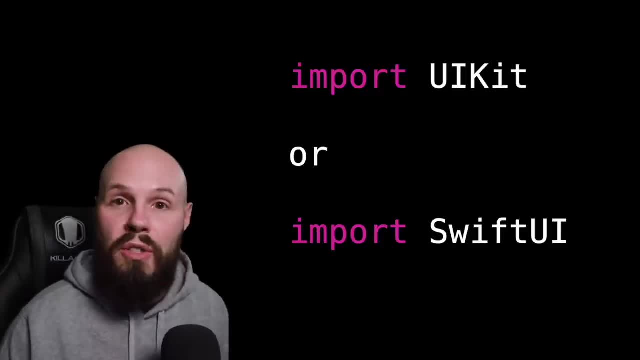 ui kit or swift ui. ui kit or swift ui- you're gonna have to know both. so in this, you're gonna have to know both. so in this, you're gonna have to know both. so in this course, uh, we focus on ui kit for the course. uh, we focus on ui kit for the. 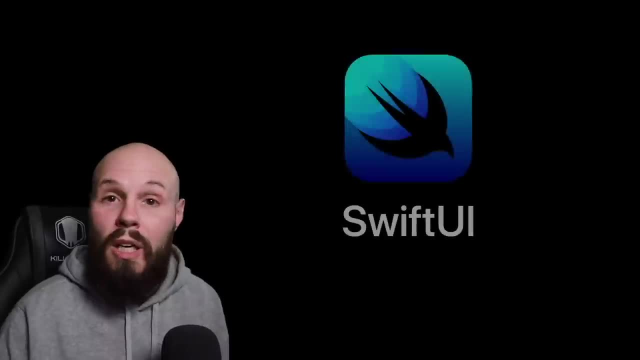 course. uh, we focus on ui kit for the most part, but i do have two videos most part. but i do have two videos most part, but i do have two videos towards the end of the course where i- towards the end of the course where i- towards the end of the course where i talk about you know what swift ui even. 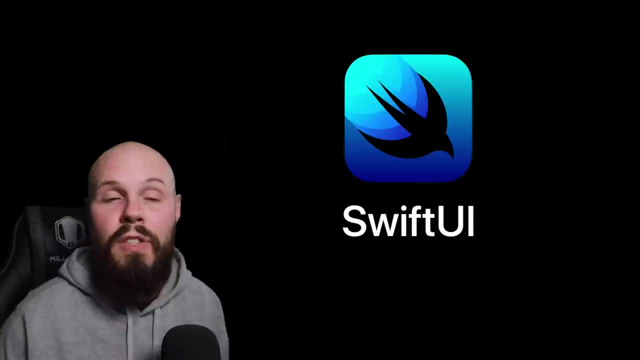 talk about. you know what swift ui even talk about. you know what swift ui even is the paradigm shift. how it's different is the paradigm shift. how it's different is the paradigm shift, how it's different from ui kit. some of the benefits you get from ui kit. some of the benefits you get. 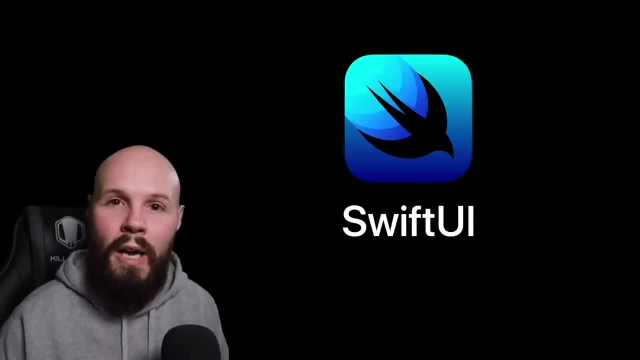 from ui kit some of the benefits you get from swift ui, and then we're going to from swift ui, and then we're going to from swift ui, and then we're going to build a pretty basic screen in swift ui. build a pretty basic screen in swift ui. 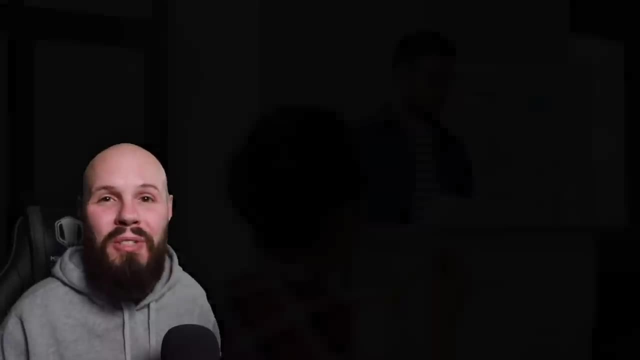 build a pretty basic screen in swift ui so you can get like a taste of how it. so you can get like a taste of how it, so you can get like a taste of how it works. but again, the entire goal of this works. but again, the entire goal of this. 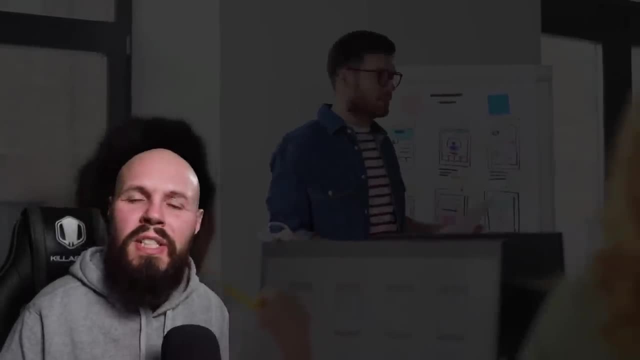 works. but again, the entire goal of this course is to expose you to this world. course is to expose you to this world. course is to expose you to this world. give you that foundation of knowledge. so give you that foundation of knowledge. so give you that foundation of knowledge so when you want to take your knowledge, when you want to take your knowledge, when you want to take your knowledge even further down, one of these paths even further down, one of these paths even further down. one of these paths. you're doing it from a good foundation. you're doing it from a good foundation. you're doing it from a good foundation. so, to sum that up real quick, you're so to sum that up real quick, you're. so to sum that up real quick, you're gonna have to learn both because we're gonna have to learn both because we're. 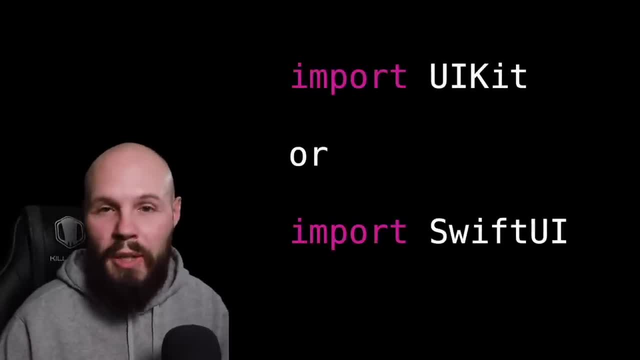 gonna have to learn both, because we're way too early in swift ui's development, way too early in swift ui's development, way too early in swift ui's development for it to be relevant in the job market, for it to be relevant in the job market, for it to be relevant in the job market and, like i said, most of you watching. 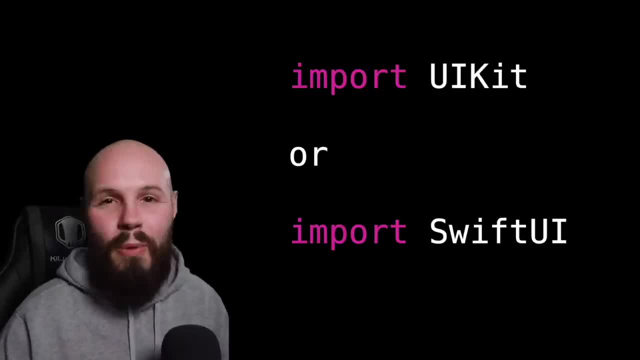 and, like i said, most of you watching and, like i said, most of you watching this are going to be in the job market. this are going to be in the job market. this are going to be in the job market within a year. swift ui won't quite be. 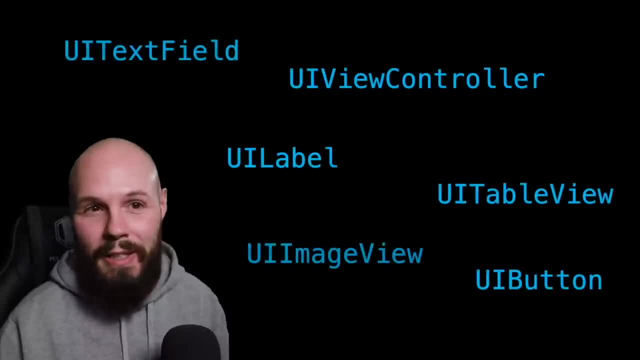 within a year, swift ui won't quite be. within a year, swift ui won't quite be ready, and even so, millions of apps are ready, and even so, millions of apps are ready, and even so, millions of apps are already in ui kit. so you're gonna have 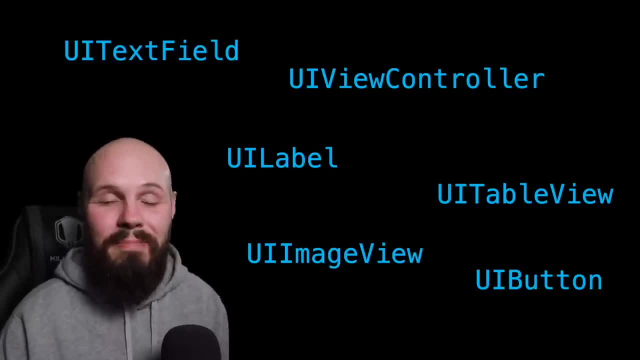 already in ui kit, so you're gonna have already in ui kit. so you're gonna have to know that it's going to be hard to to know that it's going to be hard to to know that it's going to be hard to avoid. so, unfortunately, the answer is you. 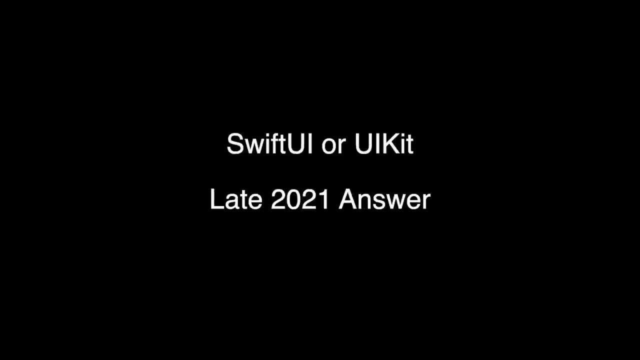 avoid so, unfortunately, the answer is: you avoid so, unfortunately, the answer is: you got to learn both and we're going to got to learn both and we're going to got to learn both and we're going to expose you to that in this course. all right, here's the updated october. 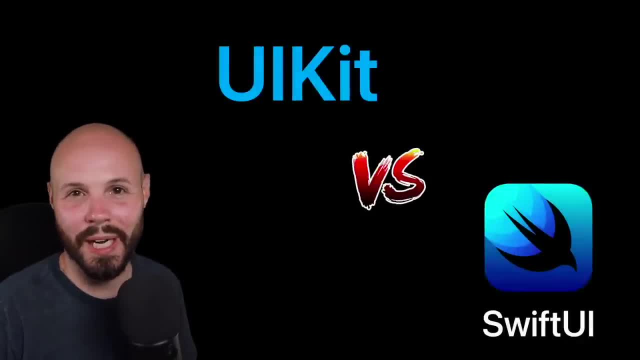 all right, here's the updated october. all right, here's the updated october 2021. opinion on ui kit versus swift ui 2021. opinion on ui kit versus swift ui 2021. opinion on ui kit versus swift ui. now i left the old video in. maybe you 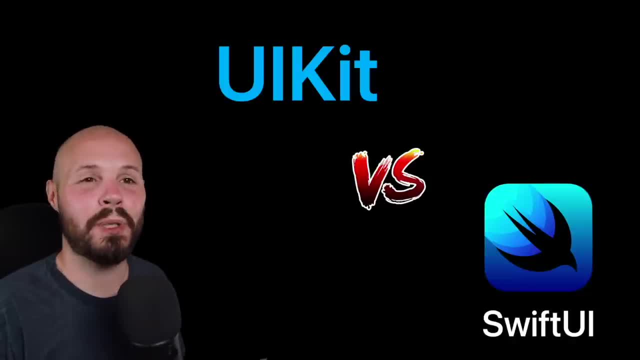 now. i left the old video in. maybe you now. i left the old video in, maybe you just watched that. just to show the just watched that. just to show the just watched that just to show the evolution of the thinking as time goes. evolution of the thinking as time goes. 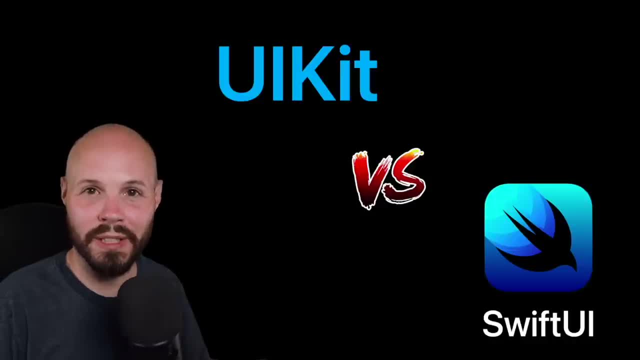 evolution of the thinking as time goes on, because that's been about a year, and on because that's been about a year, and on because that's been about a year and a half since i recorded that one and i a half since i recorded that one and i. 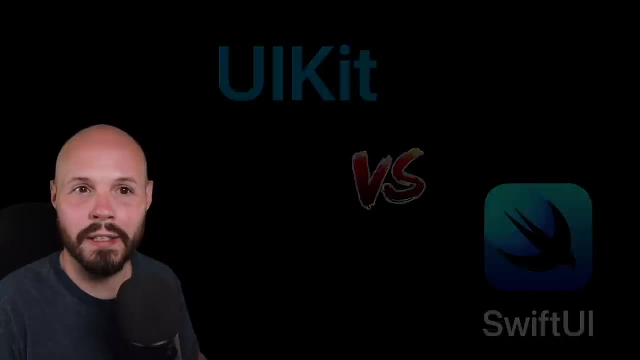 a half since i recorded that one and i said back then, you know, in two years, said back then you know in two years, said back then you know, in two years maybe swift ui would be hitting its, maybe swift ui would be hitting its, maybe swift ui would be hitting its stride. and i do believe that's true with 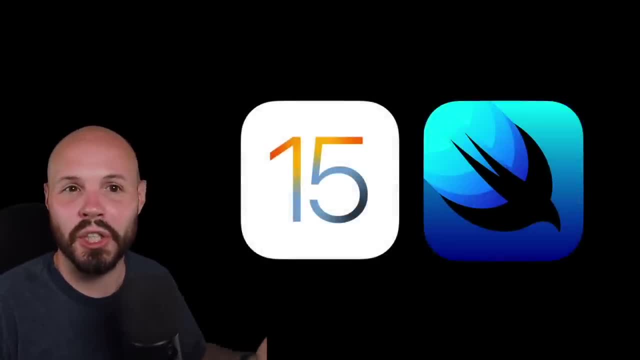 stride and i do believe that's true with stride, and i do believe that's true with ios 15. you know swift ui continues to ios 15. you know swift ui continues to ios 15. you know swift ui continues to grow and mature and i think it's. 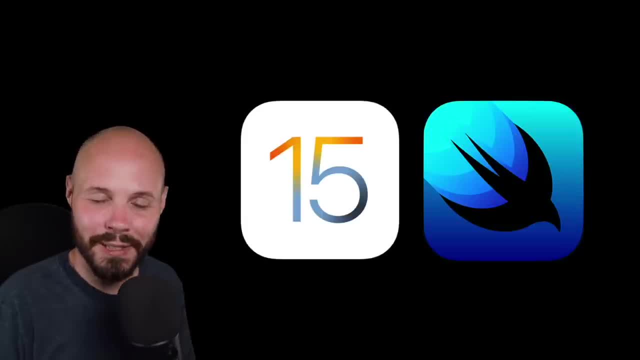 grow and mature, and i think it's grow and mature and i think it's getting there. i think it's almost there getting there. i think it's almost there getting there. i think it's almost there- not quite there yet, but it's really not quite there yet, but it's really. 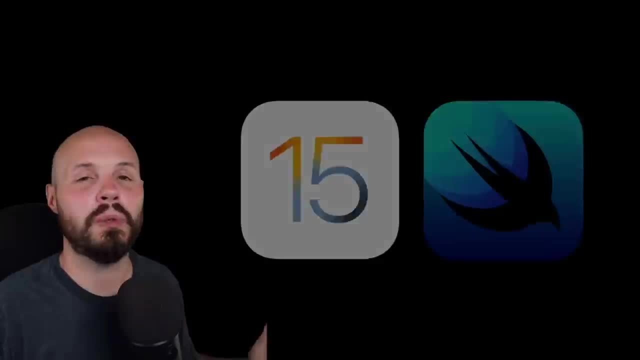 not quite there yet, but it's really getting there. but aside from getting there, but aside from getting there, but aside from functionality and the ability to build functionality and the ability to build functionality and the ability to build a great app in swift ui, a great app in swift ui. 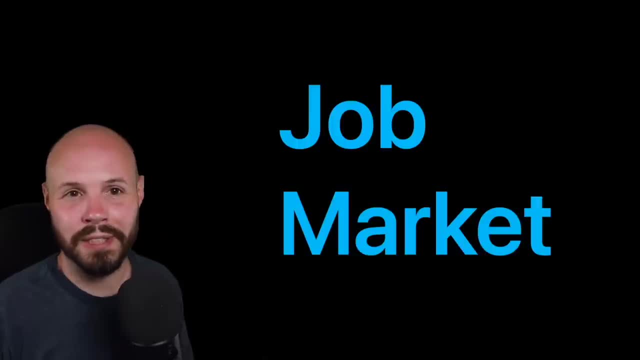 a great app in swift ui. let's talk about job market relevance. let's talk about job market relevance. let's talk about job market relevance because ui kit still dominates like i. because ui kit still dominates like i. because ui kit still dominates like i. don't know the exact percentages, but it. 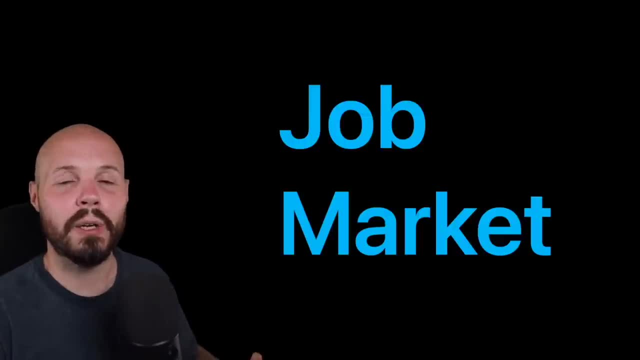 don't know the exact percentages, but it don't know the exact percentages, but it crushes it right. very small percentage crushes it right. very small percentage, crushes it right. very small percentage of jobs are in swift ui relative to ui. of jobs are in swift ui relative to ui. 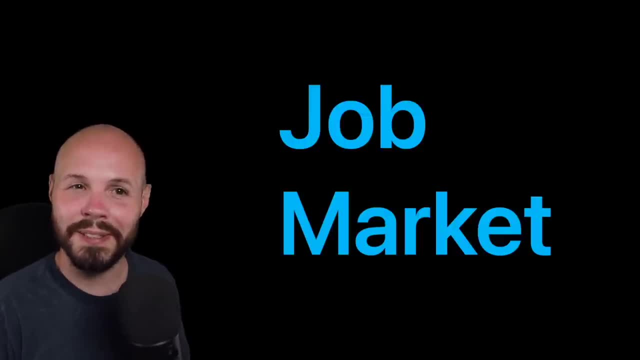 of jobs are in swift: ui relative to ui: kit still even as of october 2021, but kit still even as of october 2021, but kit still even as of october 2021. but that's starting to change, you're, that's starting to change, you're. 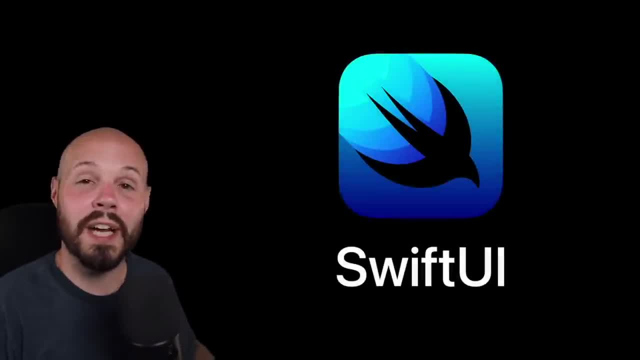 that's starting to change. you're starting to see swift ui jobs pop up, starting to see swift ui jobs pop up, starting to see swift ui jobs pop up more and more in fact. just last summer, i more and more in fact just last summer, i more and more in fact. just last summer, i hired two ios devs for a project that 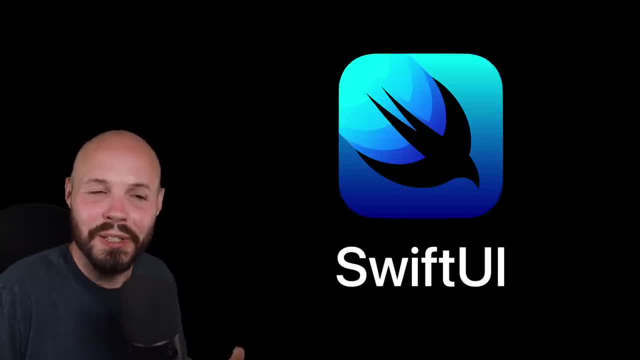 hired two ios devs for a project that hired two ios devs for a project that was completely swift ui. so again you're was completely swift ui. so again you're was completely swift ui. so again you're starting to see it, you know. starting to see it, you know. 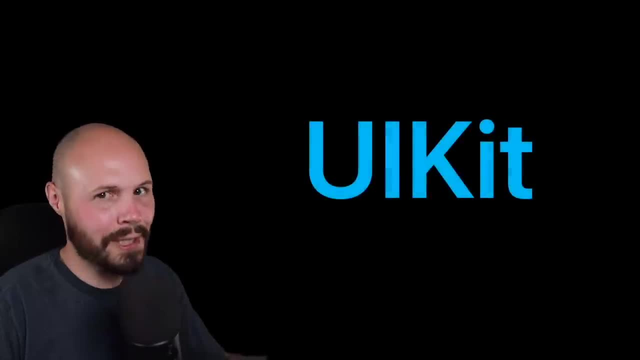 starting to see it. you know, slowly gain steam. but to be clear, ui kit slowly gain steam. but to be clear, ui kit slowly gain steam. but to be clear, ui kit still dominates as of right now. so my still dominates as of right now. so my still dominates as of right now. so my recommendation: if you're just watching, 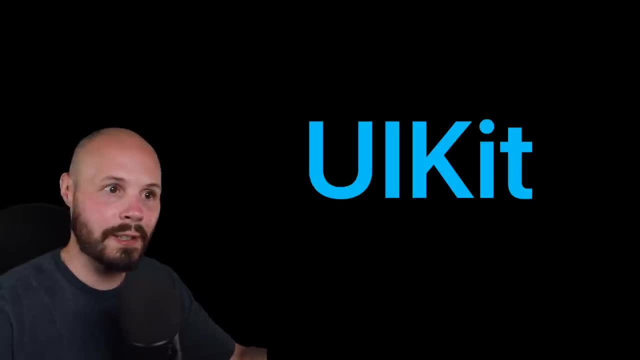 recommendation if you're just watching. recommendation if you're just watching ios dev launchpad: for the first time in ios dev launchpad, for the first time in ios dev launchpad for the first time in october 2021 or later. you're just october 2021 or later, you're just. 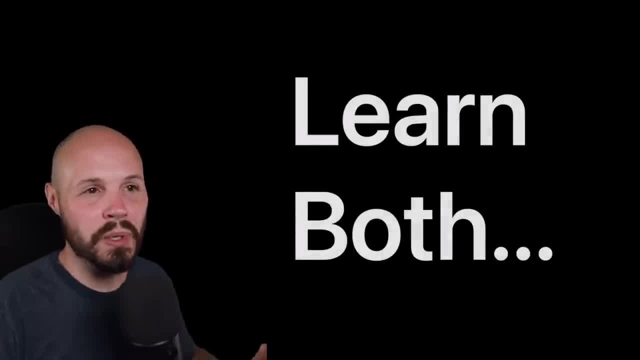 october 2021 or later. you're just getting started. uh, the recommendation on getting started. uh, the recommendation on getting started. uh, the recommendation on which to learn which to focus on. i which to learn which to focus on? i which to learn which to focus on. i would still say you need to learn both. 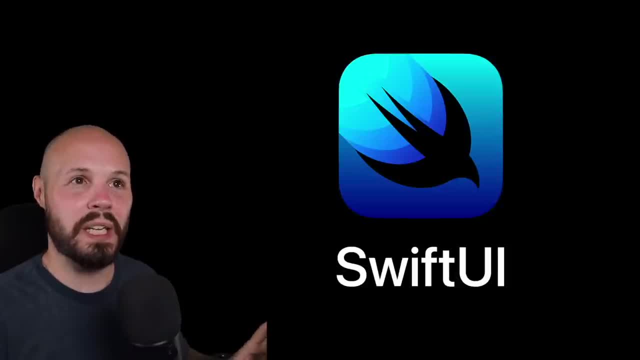 would still say you need to learn both, would still say you need to learn both. but again swift ui is picking up steam. but again swift ui is picking up steam. but again swift ui is picking up steam, for example, in the old video march of. for example, in the old video march of. 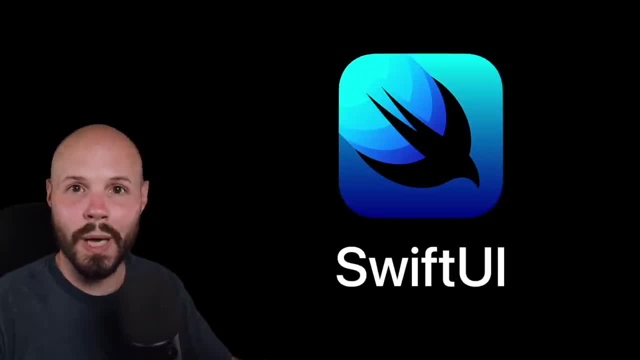 for example, in the old video march of 2020, if you were going to focus all in 2020, if you were going to focus all in 2020, if you were going to focus all in on swift ui, back then i would have said: on swift ui. back then i would have said: 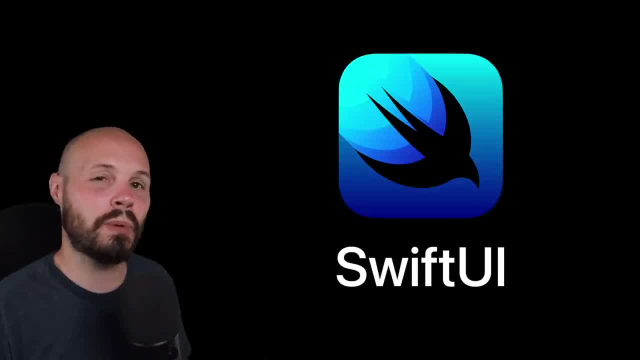 on swift ui. back then, i would have said that was a mistake. it's way too early. that was a mistake. it's way too early. that was a mistake. it's way too early. however, as of october 2021, i still think. however, as of october 2021, i still think. however, as of october 2021, i still think you need to learn both. but if someone, you need to learn both. but if someone, you need to learn both. but if someone came up to me and said you know what i'm? came up to me and said you know what i'm? 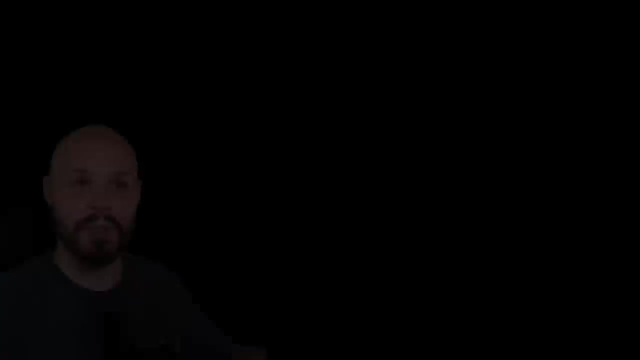 came up to me and said: you know what? i'm going all in on swift ui. this is where going all in on swift ui. this is where going all in on swift ui. this is where apple's going right- the classic wayne. apple's going right, the classic wayne. 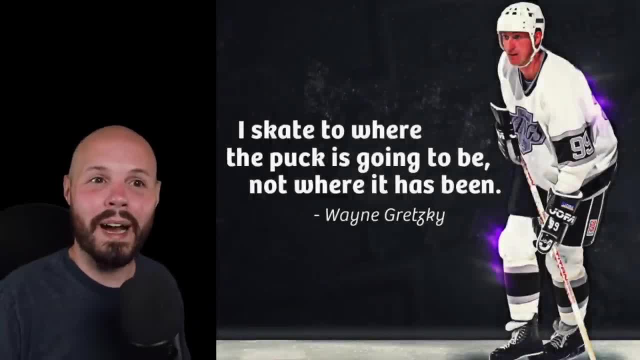 apple's going right. the classic wayne gretzky saying skate to where the puck gretzky saying skate to where the puck gretzky saying skate to where the puck is going, not to where it's been, is going, not to where it's been. 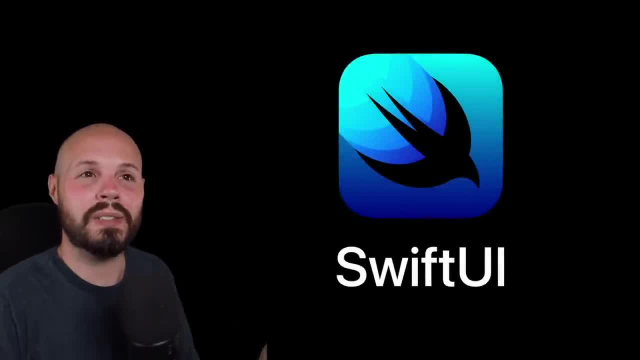 is going, not to where it's been. i probably couldn't fault you for that. i probably couldn't fault you for that. i probably couldn't fault you for that because, again the process of going on, because again the process of going on, because again the process of going on this journey of becoming an ios. this journey of becoming an ios, this journey of becoming an ios developer, typically takes six months to developer, typically takes six months to developer typically takes six months to two years. so if you won't even hit the two years, so if you won't even hit the two years, so if you won't even hit the job market for 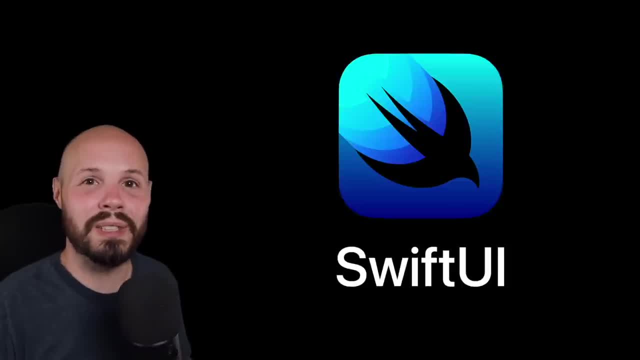 job market for job market for six months to even two more years. from six months to even two more years. from six months to even two more years from now. yeah, i think swift ui is gonna now. yeah, i think swift ui is gonna now. yeah, i think swift ui is gonna gonna look a lot better. however, i would 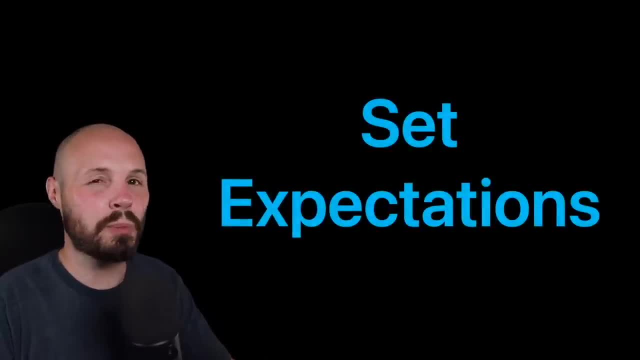 gonna look a lot better, however. i would gonna look a lot better. however, i would want to set your expectations, want to set your expectations. want to set your expectations that ui kit will still probably be that ui kit will still probably be. that ui kit will still probably be dominant. so you are going to be. 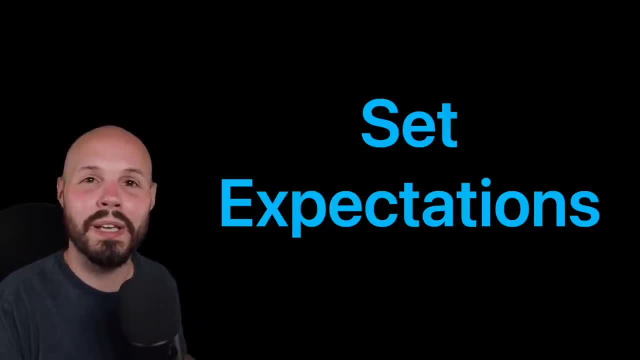 dominant. so you are going to be limiting your, your job prospects, limiting your, your job prospects, limiting your, your job prospects, but it still may be the right move for, but it still may be the right move for, but it still may be the right move for the future. quick example: that's what i 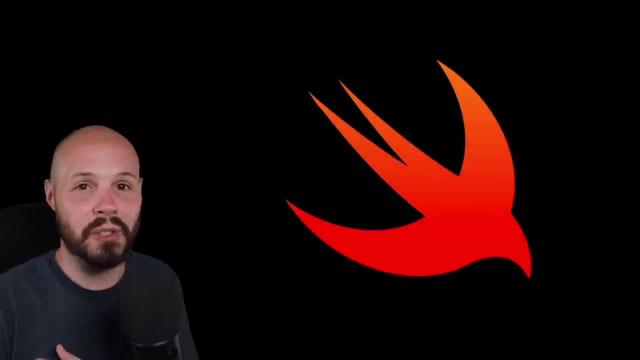 the future quick example. that's what i. the future quick example. that's what i did with swift- swift came out in 2014. did with swift- swift came out in 2014. did with swift- swift came out in 2014. it's about the time i started learning. it's about the time i started learning. it's about the time i started learning and, to be honest with you, swift is what? and to be honest with you, swift is what? and to be honest with you, swift is what got me into ios development. got me into ios development. 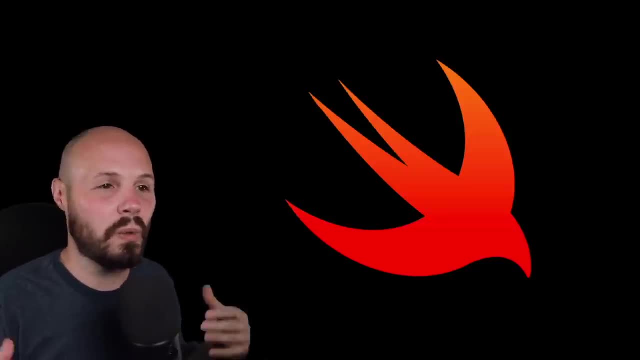 got me into ios development and i said that day because it was the and i said that day because it was the. and i said that day because it was the same situation, objective c. same situation, objective c, same situation, objective c was still dominant. no jobs were in swift. was still dominant. no jobs were in. swift was still dominant. no jobs were in swift. but i said that i was like you know what. but i said that i was like you know what, but i said that i was like you know what. it's going to take me two, three years to. it's going to take me two, three years to. it's going to take me two, three years to be really good at this. be really good at this, be really good at this. so again, i want to go to where apple's. so again i want to go to where apple's. 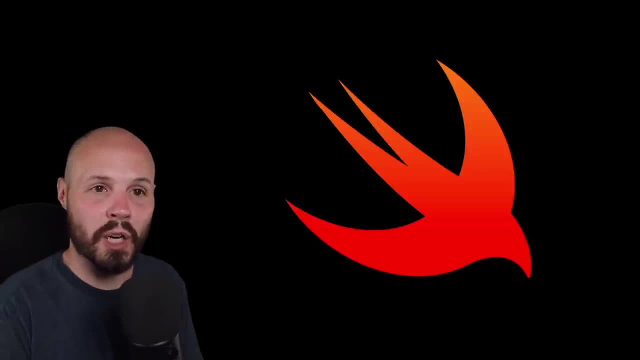 so again, i want to go to where apple's going. so i went all in on swift going. so i went all in on swift going. so i went all in on swift, knowing that would limit my job, knowing that would limit my job, knowing that would limit my job prospects. because objective c was. 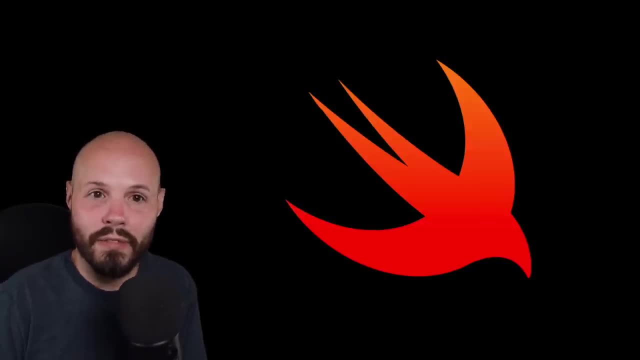 prospects because objective c was prospects, because objective c was everywhere, everywhere, everywhere. but you know, i worked at it for a year. but you know i worked at it for a year. but you know, i worked at it for a year or so and finally got that swift job and or so, and finally got that swift job and or so, and finally got that swift job. and i've been focused on swift, i've been focused on swift, i've been focused on swift day one and i think that was a good move- day one, and i think that was a good move. 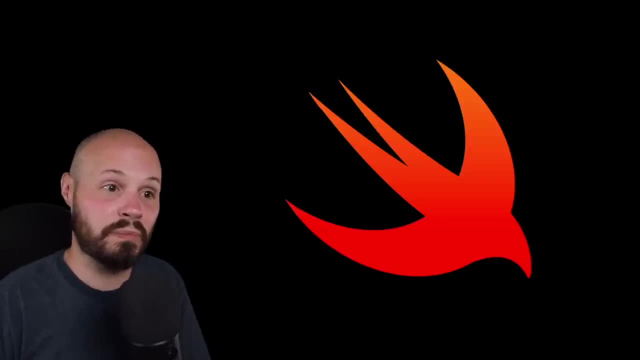 day one, and i think that was a good move. here we are, you know six, seven years. here we are. you know six, seven years. here we are, you know, six, seven years later, and i've been writing swift later and i've been writing swift later and i've been writing swift pretty much 100 from day one, so that pretty much 100 from day one. so that, pretty much 100 from day one. so that has benefited me. so i think has benefited me, so i think has benefited me. so i think, at this point in time, if you were to go, at this point in time, if you were to go, 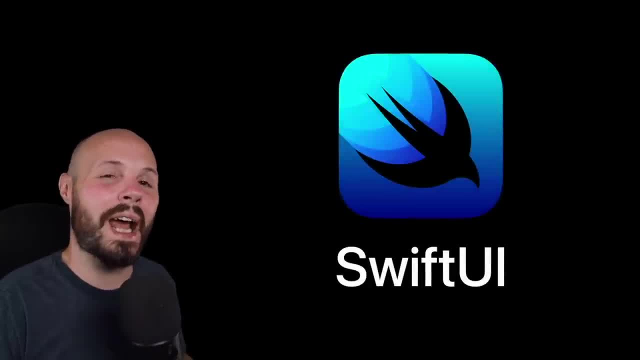 at this point in time, if you were to go all in on swift ui, all in on swift ui, all in on swift ui, i think a similar thing might happen. i think a similar thing might happen. i think a similar thing might happen there. so again, to be clear: ui kit is there. so again to be clear: ui kit is there. so again to be clear: ui kit is still dominant as of now. it will still still dominant as of now. it will still still dominant as of now. it will still be dominant a year from now. be dominant a year from now. 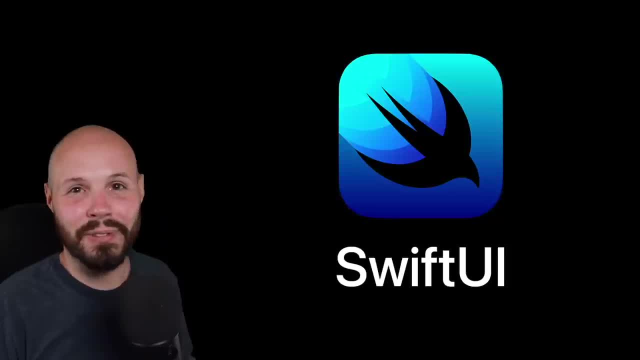 be dominant a year from now? uh. but if you were to go on swift ui? uh. but if you were to go on swift ui? ah, i couldn't fault you as long as you, ah, i couldn't fault you as long as you. ah, i couldn't fault you as long as you set your expectations. 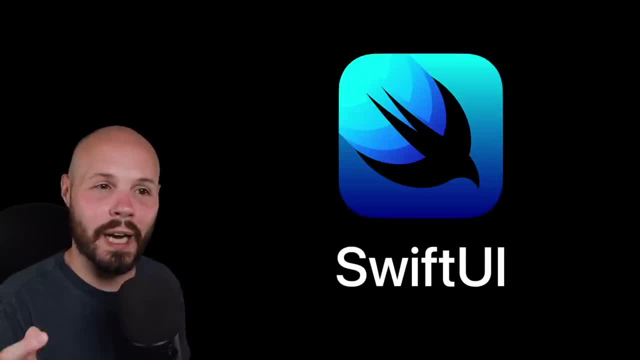 set your expectations. set your expectations that it may be a little harder to find. that. it may be a little harder to find. that it may be a little harder to find a job, but if you can find one, uh, it'll a job. but if you can find one, uh, it'll. 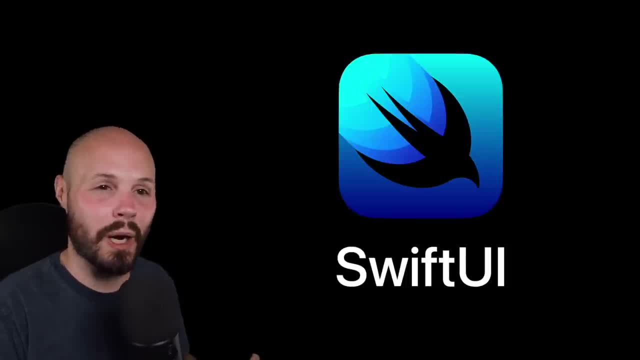 a job, but if you can find one, uh, it'll really benefit you. that you kind of made really benefit you. that you kind of made really benefit you that you kind of made that gamble, that leap on swift ui, that gamble, that leap on swift ui, that gamble, that leap on swift ui early. so there you go. that's the updated. 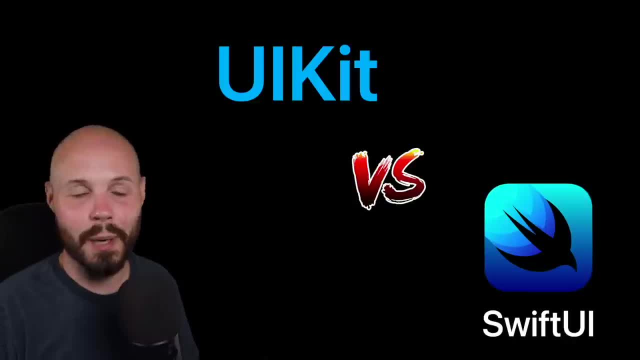 early. so there you go. that's the updated early. so there you go. that's the updated opinion. to sum it up, you still need to learn both. UIKit is still going to be dominant for a couple more years, But for those of you that like to be a little risky, like to take chances, I wouldn't fault. 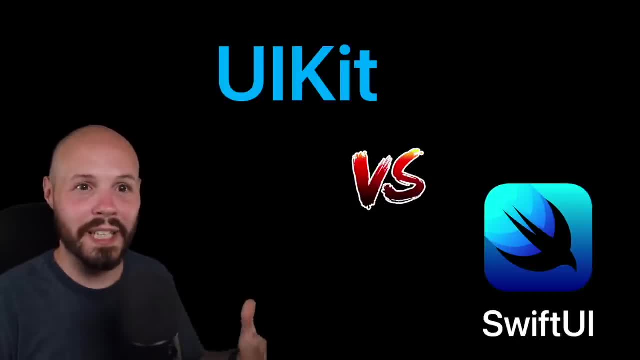 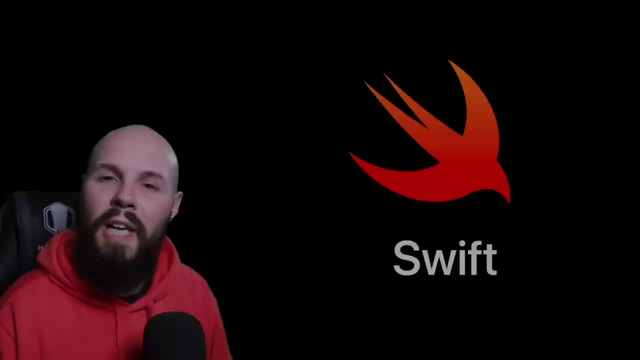 you for going all in on SwiftUI, But if you are more conservative, you are worried about landing a job right away. maybe you should focus on UIKit. Before we actually start writing Swift code, let's talk about what Swift is and give you a brief history. right, It's good to know. 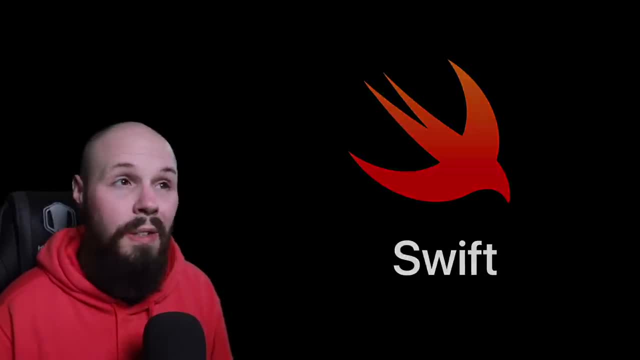 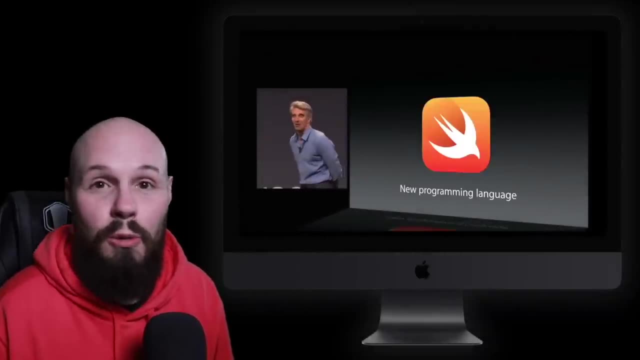 what's going on with the language before you start learning. So Swift is relatively new. It was a surprise announcement at WWDC back in 2014.. Like, developers had no clue it was coming. they're watching the announcements and it's like holy crap, a whole new language Like 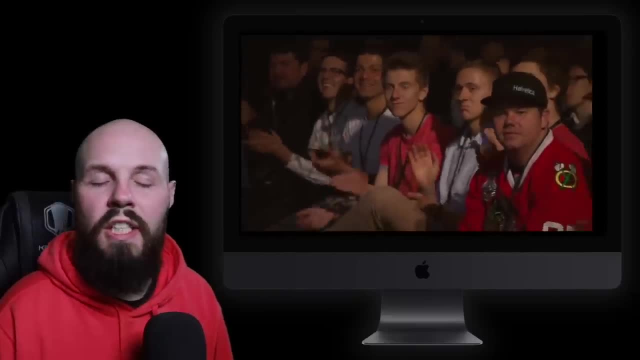 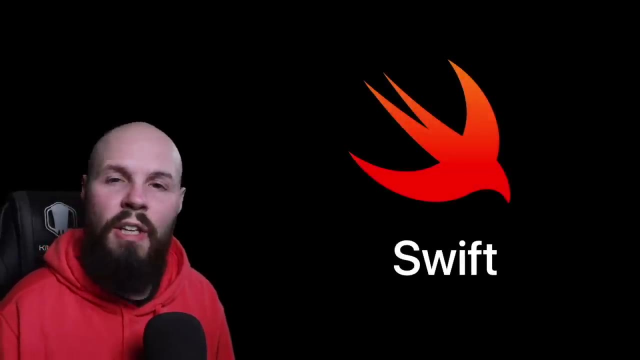 everything changed back in 2014, when Swift was announced. What the engineers at Apple did was they took all their previous knowledge with Objective-C and everything, because Objective-C is, you know, 30 years old and they did all their research on the new and modern languages. 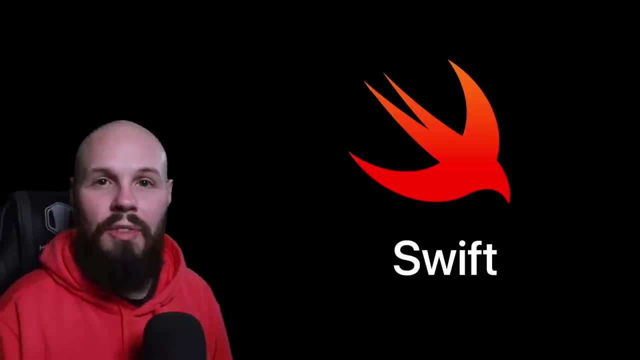 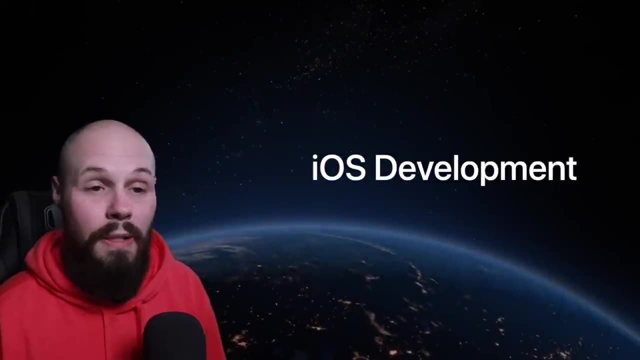 and where things were going and they took all that and they built Swift, Apple's next generation programming language that is for their future. Now a lot of people always ask me: you know, because native iOS development? admittedly it is a niche programming language, It's not as widespread as you know, Java or 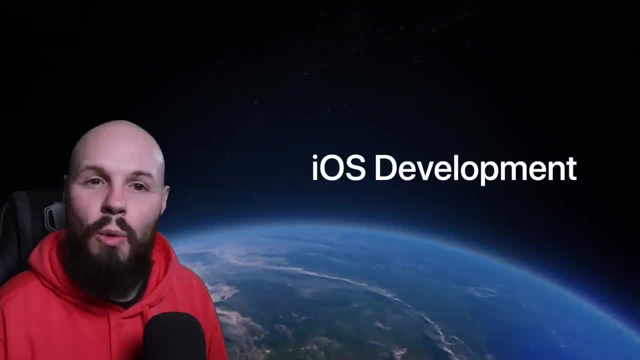 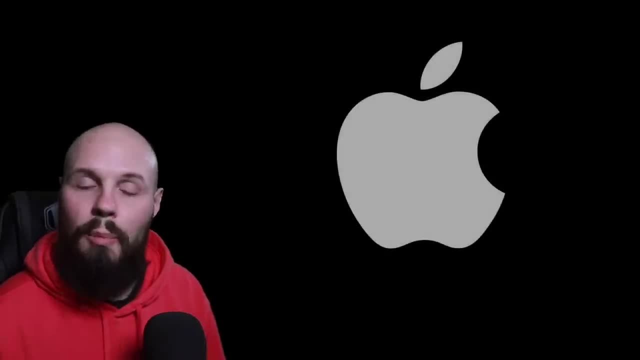 JavaScript or Python, but it is niche. So a lot of people ask me, like, if I become an iOS developer, like, does that limit my career choices? And I always say, like, as a Swift developer, iOS developer, whatever you want to call it, you're tying your career to Apple And as long as you. 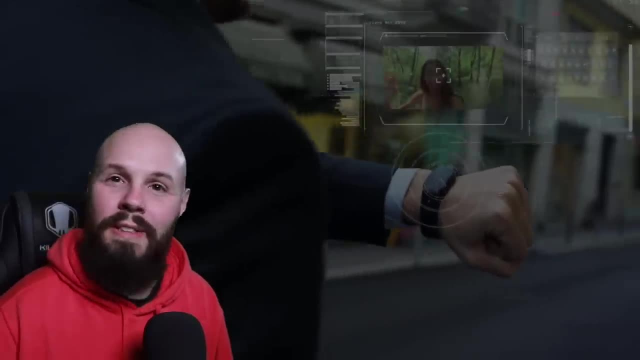 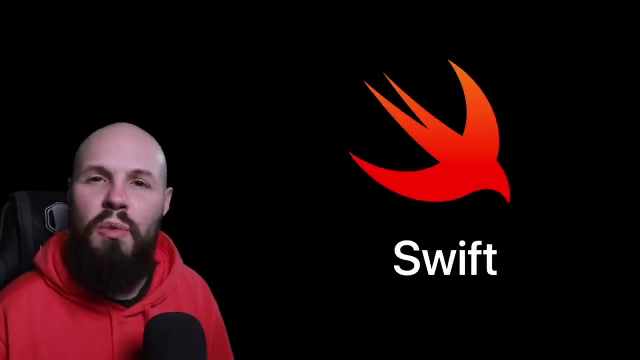 believe that Apple's not going anywhere and it's going to be around for a long time, you know, into AR VR. whatever direction they go, it's a pretty safe bet. Speaking of safety, amazing segue, one of Swift's major selling. 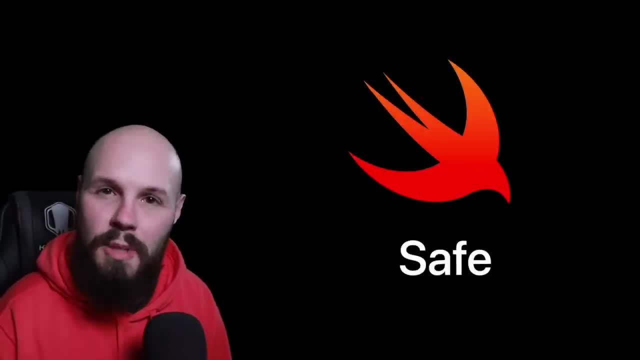 points is it's just a safe language. There's type safety objects you know can't be nil unless you use optional. Basically, a big thing of Swift is you want to have a lot of compile time errors, not runtime errors. As a new programmer, newly aspiring programmer, that 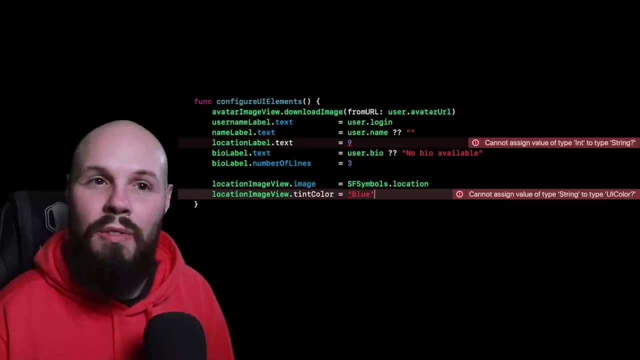 may have meant nothing to you. Basically, what that means is Swift tends to give you errors at the time of writing your compode or when the code compiles in Xcode, whereas runtime errors are. you don't know about the error until the app crashes. Then you got to debug, So you're. 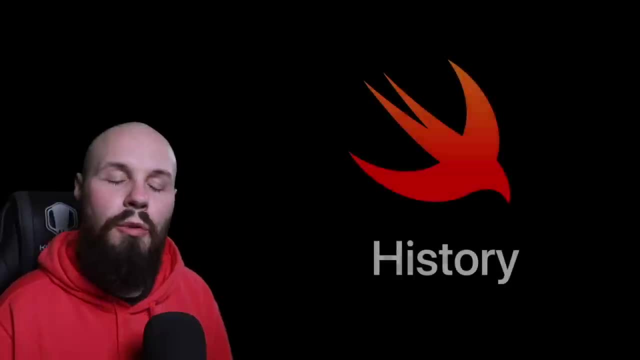 going to see a lot of compile time errors before you can even build your app with Swift. Let's run through Swift's very brief history Again. it was announced in 2014, just to let you know kind of how Swift has evolved over the past couple years Now. Swift had some massive changes and very 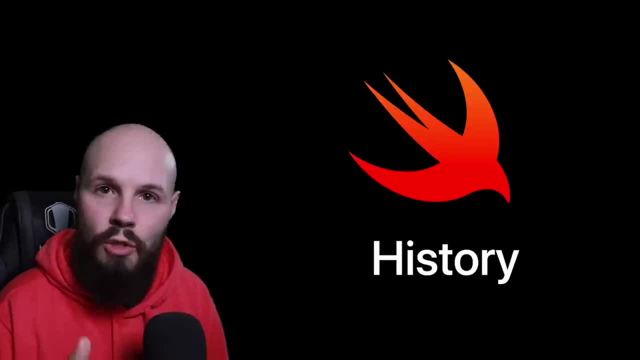 rapidly in its early days, And the reason you should know this as a new beginning Swift developer is because, if you look for a blog post or maybe a stack overflow answer or some resource that is old and hasn't been updated since, you know, 2015,, 2016,. that can get you in a lot of trouble Because again through 2014,, 15,, 16,, 17,. Swift has changed a lot, But the good news is that change is starting to slow and Swift is slowly starting to mature. All right back to the beginning, Like I said. 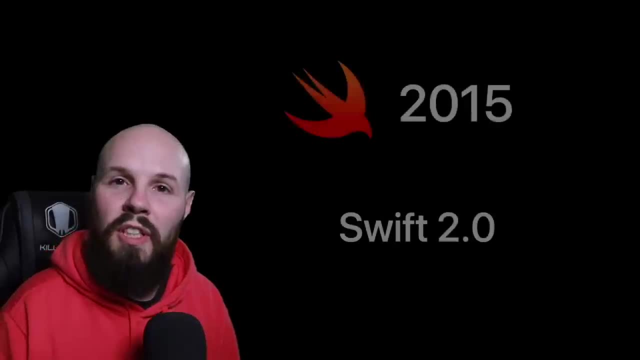 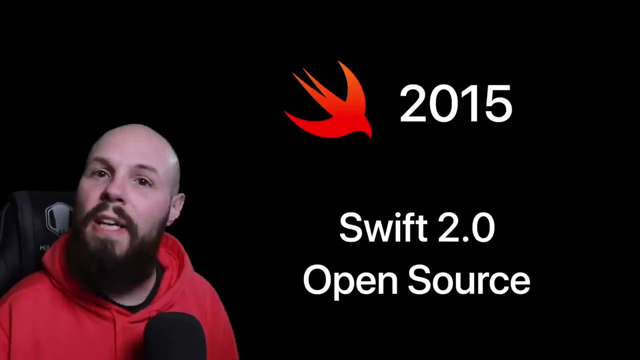 before. it was a surprise announcement in 2014.. By 2015,, Swift 2.0 was announced And it was also announced that WWDC in 2015, that Swift was going to go open source later that year. it ended up. 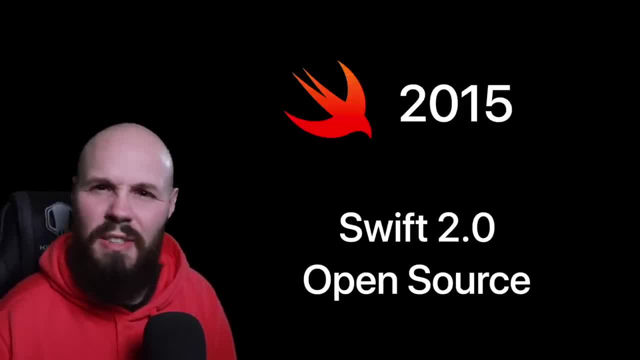 going open source and Swift 2.0 was going to go open source. So Swift 2.0 was going to go open source and Swift 2.2 later, like in December of 2015.. Now, open source was a big deal because 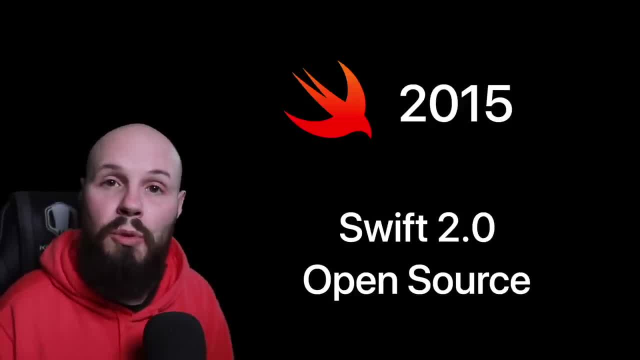 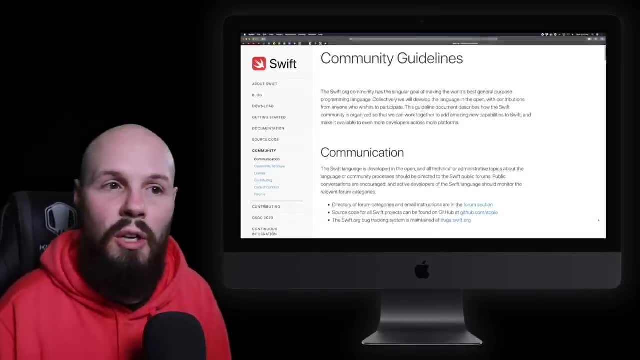 that meant the iOS developer community as a whole could contribute to Swift language itself. If you ever want to look into this, go to swiftorg. you can see the forums and see the discussions on proposals that are going to be implemented into Swift. Now don't get me wrong. this is like 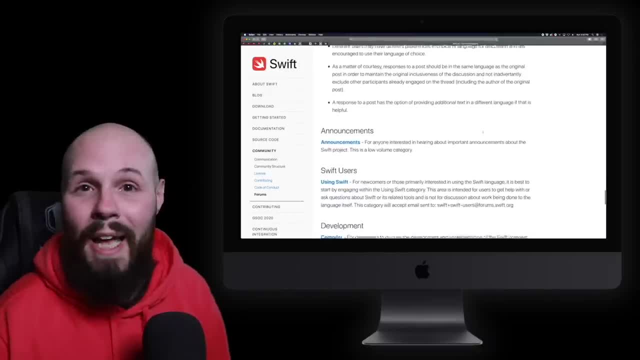 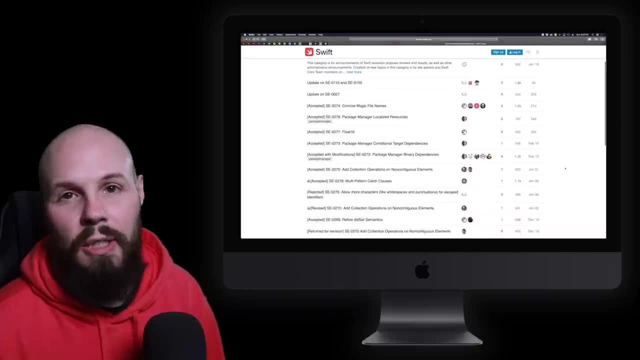 heavy language implementation details. most of it's even over my head, But if you are interested in, like, how the language gets built or you know what new things are coming to the language, that's the spot to go. look, Now going. open source was a big deal, But in 2016, Swift 3.0 came out. 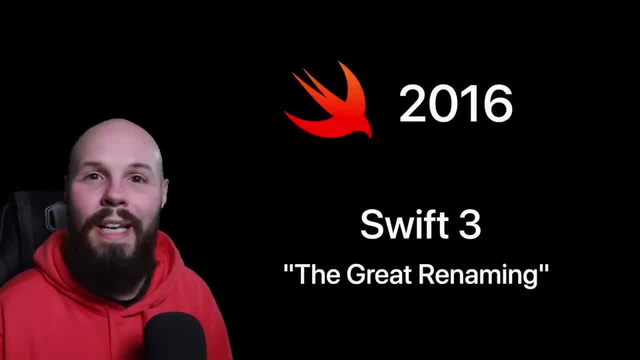 And that was a huge deal. That was dubbed the great renaming. Basically, what happened between Swift 2.0 and Swift 3.0 was a ton of breaking changes in Swift's API. So it was a nightmare converting a Swift 2.0 codebase to a Swift 3.0 codebase because so much broke and so much changed. 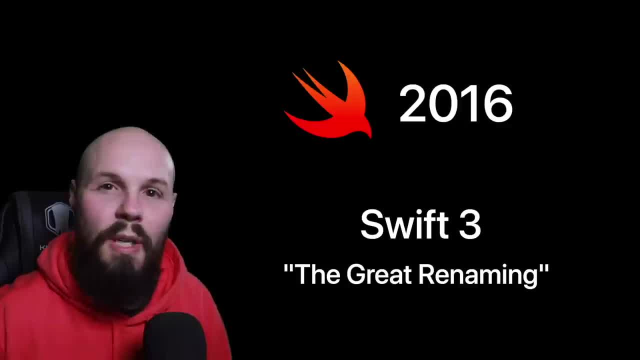 However, Swift 2.0 to Swift 3.0 was kind of like just ripping off the bandaid right. It was a ton of pain right there And it was a lot of work And it was a lot of work, And it was a lot of work And you know, Swift 3.0 to Swift 4.0, Swift 4.0 to Swift 5.0, and upcoming Swift 5.0 to Swift 6.0 have been a breeze compared to that. So they kind of got all the pain out of the way going from Swift. 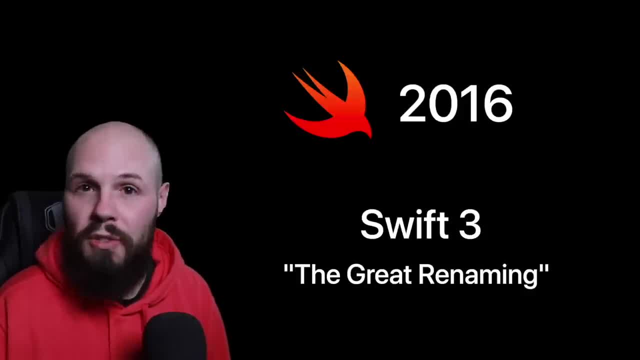 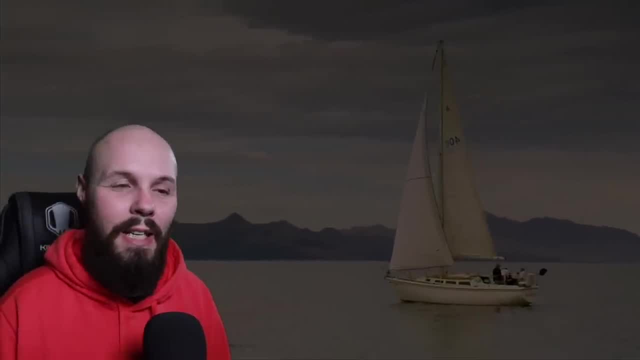 2.0 to Swift 3.0. So again, when you're looking at old resources or old blog posts, if it was done in Swift 2.0, stay away from it. But like I said, after that major Swift 3.0 pain, it's been smooth. 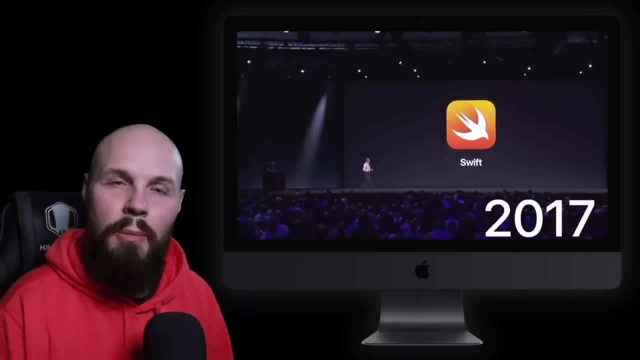 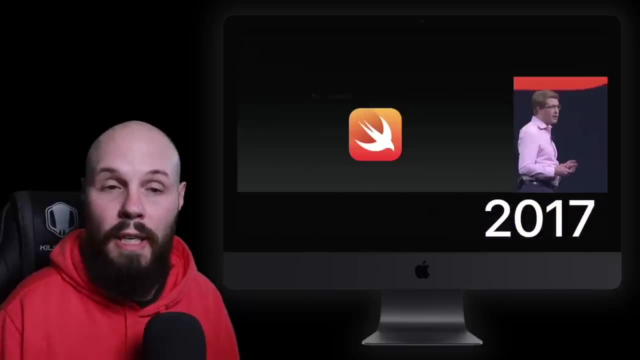 sailing since then. Swift 4.0 came out in 2017.. But Swift 4.0 kind of was the last major number release at WWDC Up until Swift 4.0, again every dub dub, which was June of every year. 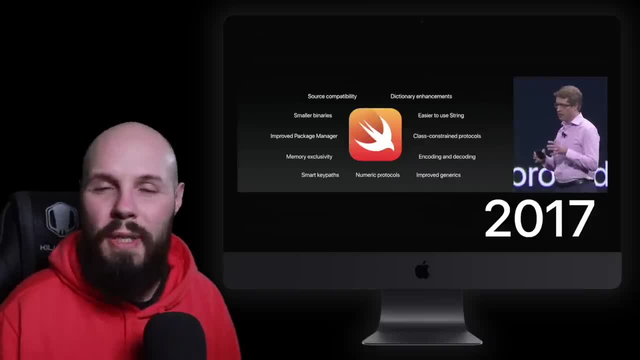 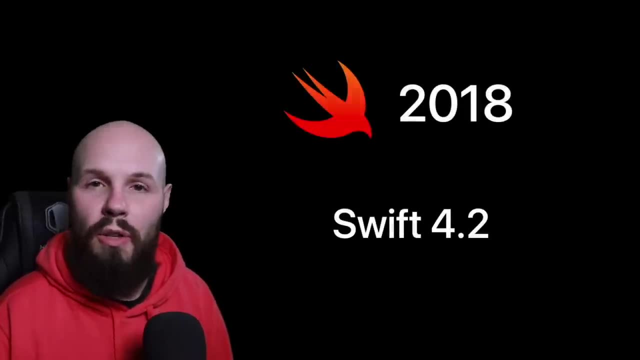 we would get a new Swift, Swift 3.0, Swift 4.0.. Well, they've kind of slowed down since then And you know, WWDC 2018 was Swift 4.2.. It has slowed down And they recently announced with: 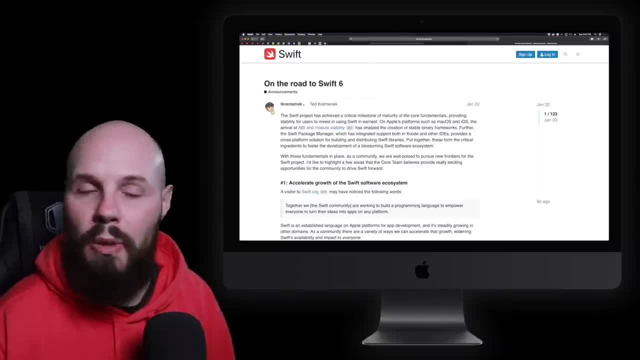 on the roadmap to Swift 6.0 that you know there's no major year release, It's just going to release when it's ready, which is great. I love that, because it almost felt like they were rushing features into the language to make the annual release cycle. 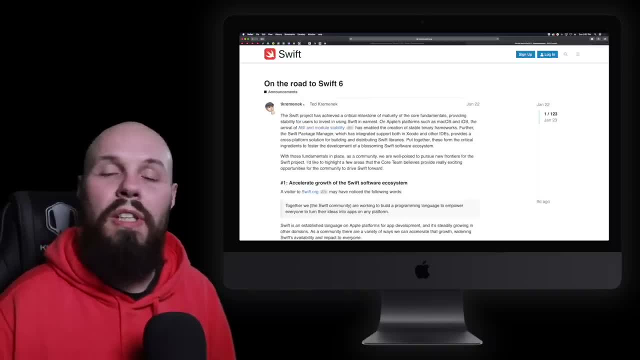 And you know they've kind of learned and said: you know what Swift 6.0 will release when it's ready. No release date. It'll come Again that, along with the fact that you know the changes. 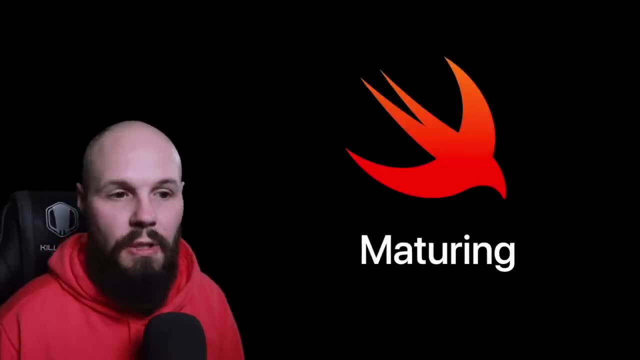 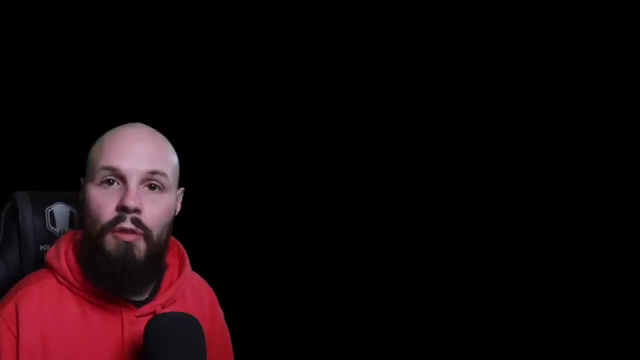 coming aren't major breaking changes shows that the language is maturing And because the language is maturing, we're starting to see it leak out into non-Apple native platforms. For example, machine learning at Google via TensorFlow. that is done in Swift now. That's in part two. 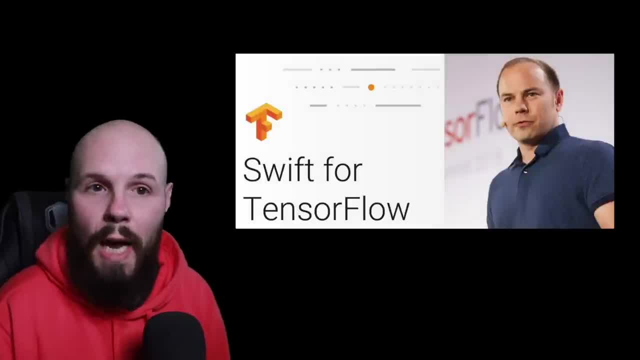 Chris Lattner, who is one of the main developers behind creating and launching Swift at Apple. Chris Lattner, who is one of the main developers behind creating and launching Swift at Apple. He has since left Google as well- just recently- but he was spearheading Swift at Google as well. 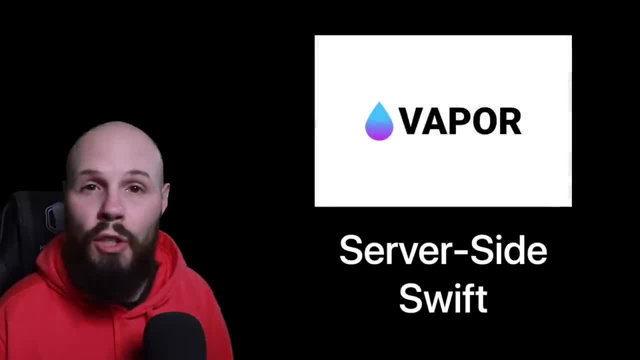 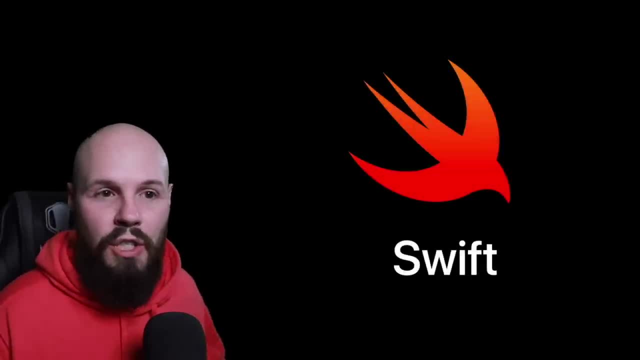 So you know it got a good foundation over there And now you can also write server code in Swift. Swift is almost ready for Windows. That's being actively worked on. But again, Swift is such a young language that you know it may not be on all these other platforms yet, but you can start. 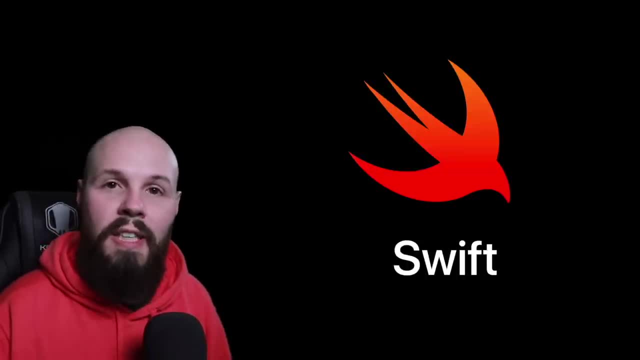 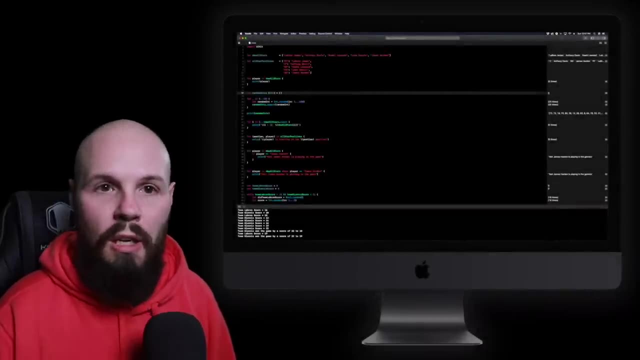 to see the beginnings of it And if you kind of fast forward your mind five to 10 years, it's looking pretty good. I want to go into a bunch of videos about the basics of the Swift language. I want to reiterate that these are just high level videos. right, A lot of these topics could be almost whole courses. 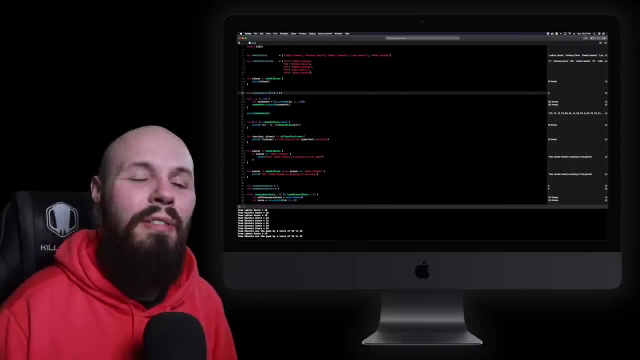 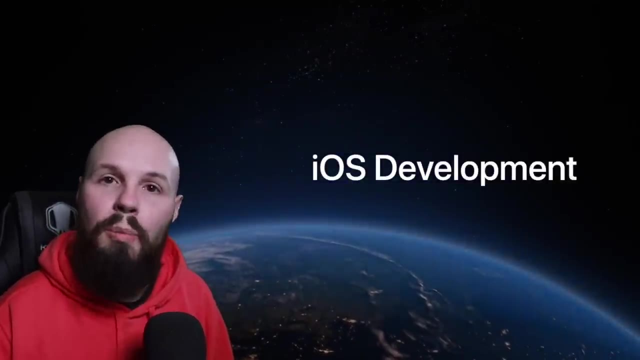 in and of themselves, or at least multiple, 10, 15 minute videos. Again, like I said before, this is supposed to be your first video, just your exposure to this world. So again, these topics will be pretty high level, but it is a good foundation for your future learning. 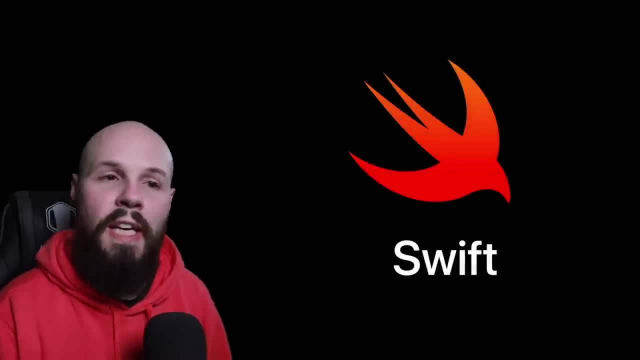 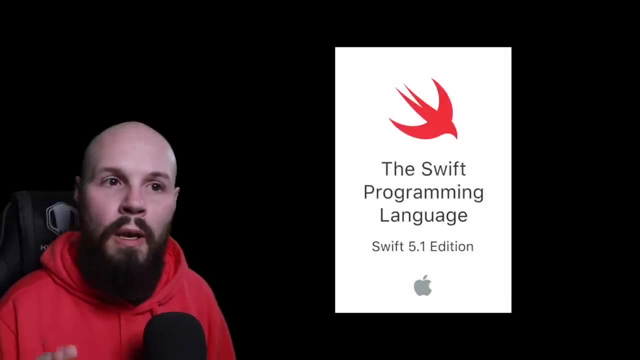 Speaking of future learning, I want to recommend a couple of resources for you to check out. to again just expand. First is the Swift programming language book directly from Apple. A little bit of a warning, and we're going to talk about this later in the books video, But this is basically Apple's. 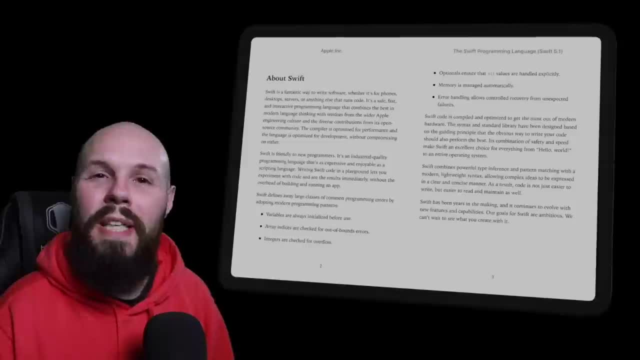 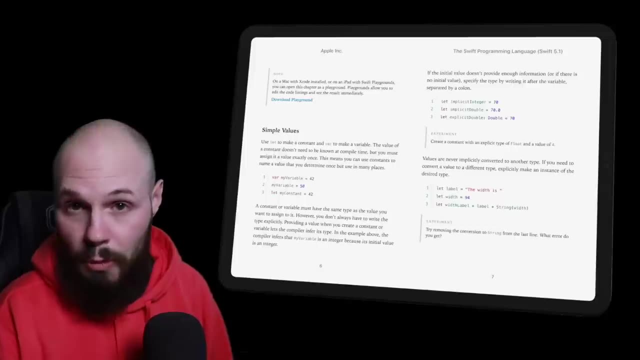 instruction booklet for Swift, So it is pretty technical. I remember reading it as somebody who had never coded before and just started my Swift journey, which may be exactly where some of you are at. It was way over my head, but it is a very valuable piece of information, So I do recommend. 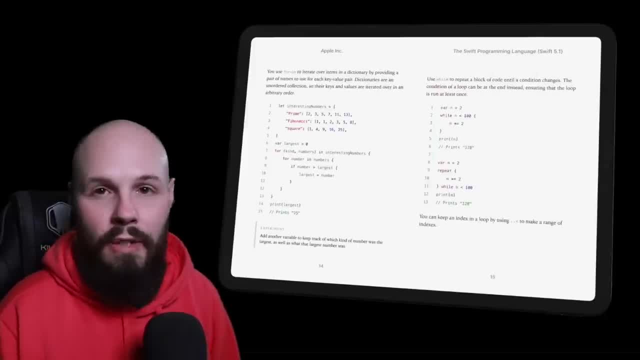 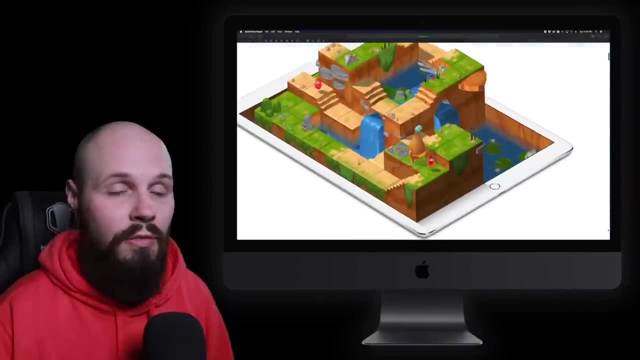 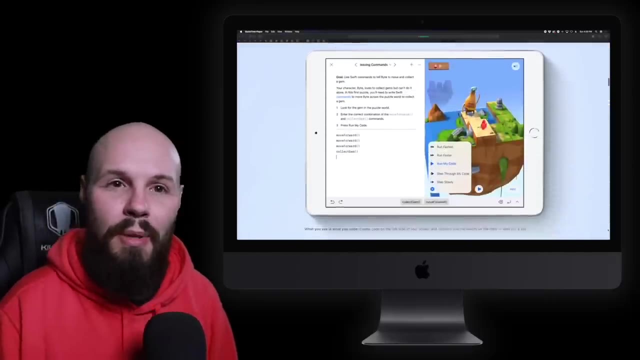 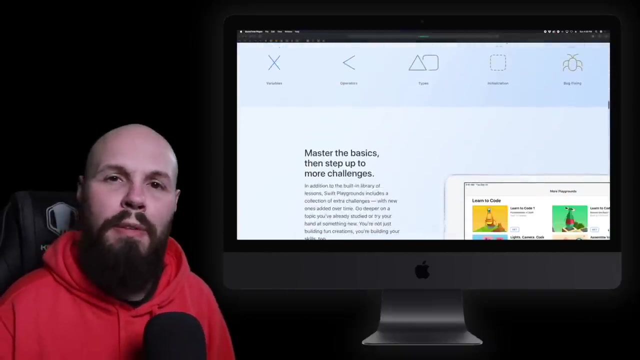 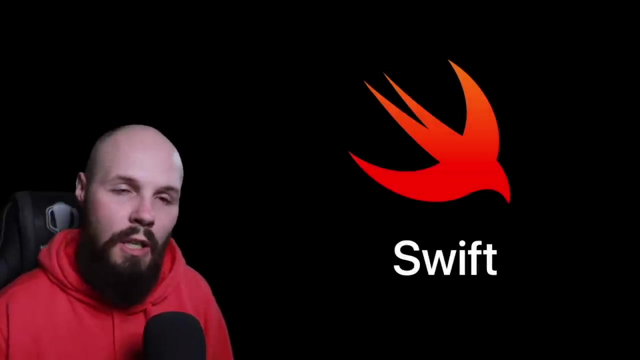 at least checking it out. But again, don't forget to check it out And I'll see you in the next video. Thanks for watching and I'll see you in the next video. Bye Overview. And then another is a pretty fun video about the reveal of Swift at WWDC in 2014.. And you 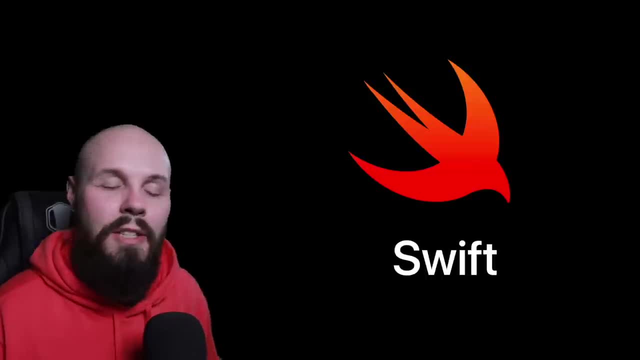 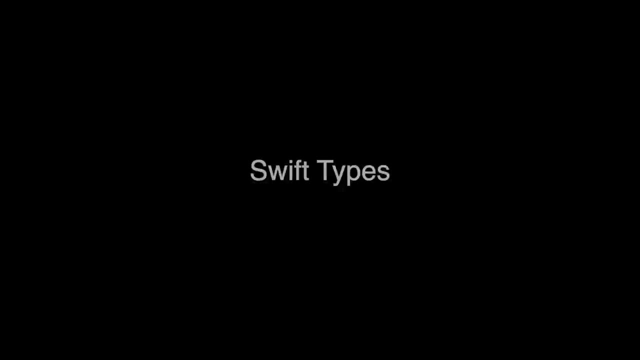 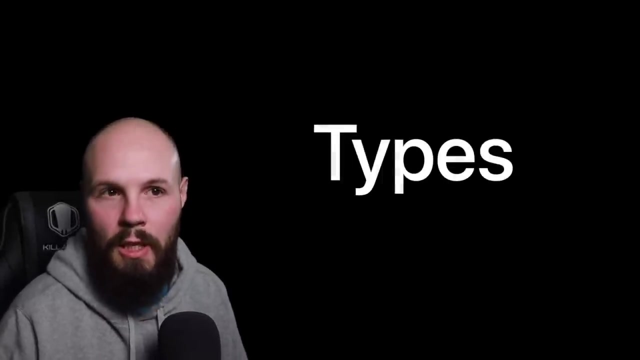 can hear, like the gasps in the audience. It's pretty cool to go back and watch. So that's a brief history of Swift. Let's start writing some code. Let's talk about a foundational concept in Swift, and that is types. What is a type? It's what type. 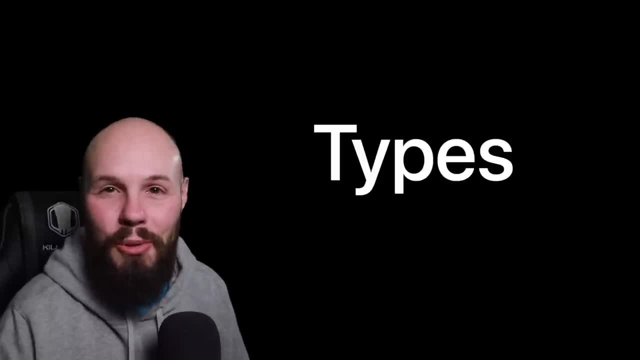 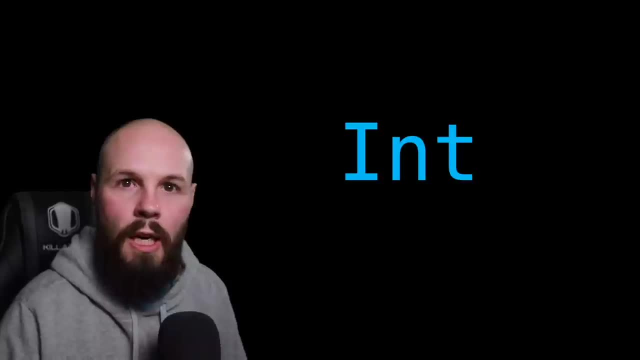 something is Great explanation, I know. Let me show you and that'll make more sense. In this example we're talking about the type int, which is short for integer, which is a whole number. Now it can be negative, But an example. 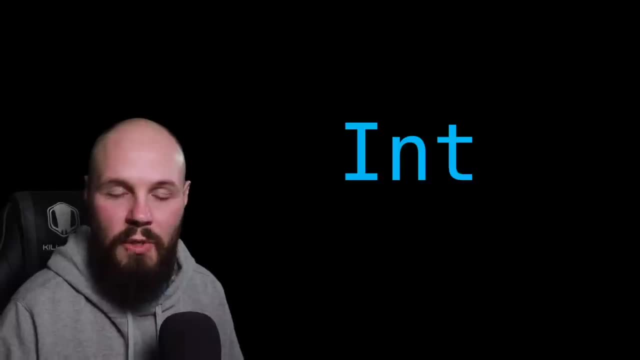 of that is, let's say, you have a high score in a video game. So we're going to create a variable called high score. It is of type int and it equals zero. right, We're not very good at the game, But the type is int. So what we're saying is this: zero is an integer. Now in Swift there's 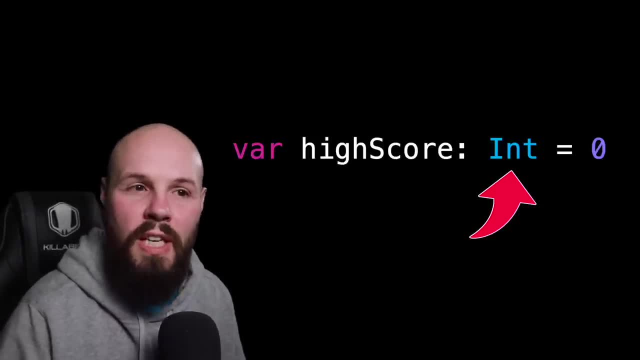 tons of different types. We're going to talk about the foundational one and then we're going to talk about the ones in this video, But the general idea is that our variable high score is of type int and it is equal to zero, which zero is an integer. Let's build upon that numerical example and talk. 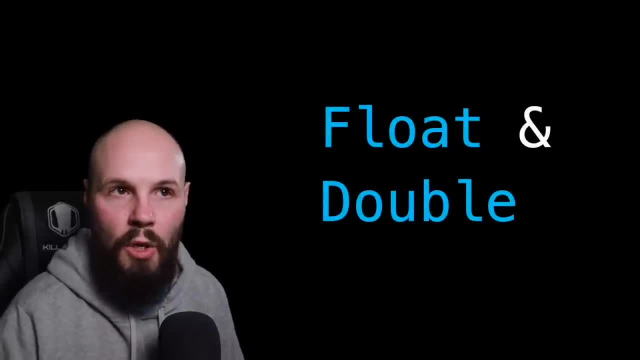 about our next two types, and that is float and double. Whereas if integer was a whole number, float and doubles are decimals. Now, the main difference you need to know between float and double is the amount of decimal places, or the precision. A double has a precision of at least. 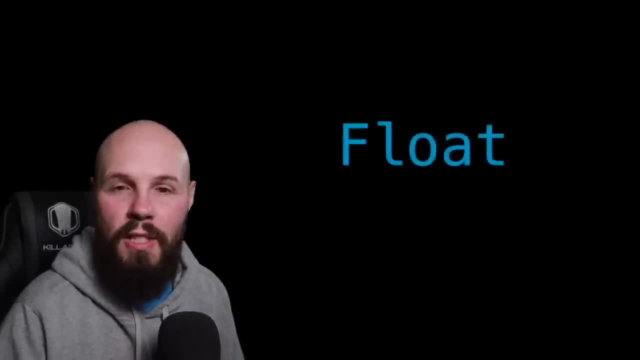 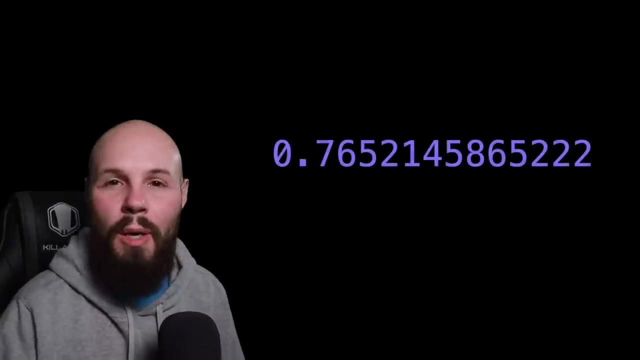 15 decimal places, so pretty long. A float has a precision of at least six decimal places. So, as you can tell, a double is more precise than a float. And now, with these floats and doubles, you don't have to use all these. 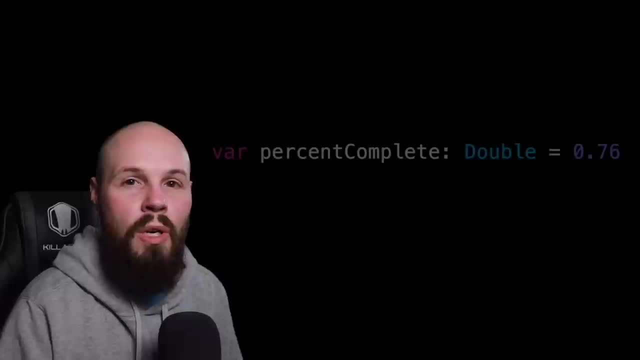 decimal places. That's just their capabilities, As you'll see in this example of a percentage complete. like we want 76%, So we'll just do 0.76, right, You don't have to use all those decimals. 0.76 gets the message across. But to reiterate here we have our variable called percentage. 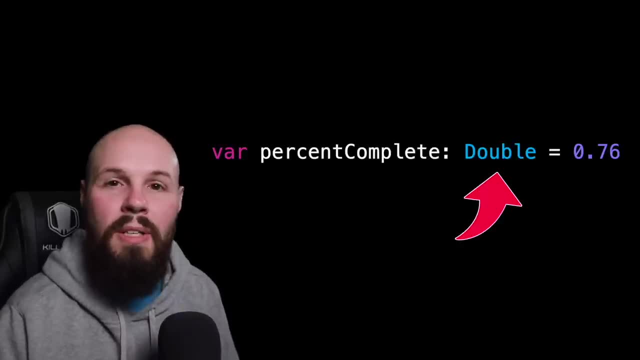 complete and that is of type double and it equals 0.76.. Moving away from the decimal place, we're going to take a look at the percentage complete. Moving away from our numerical examples, we have string. Now string represents text And in: 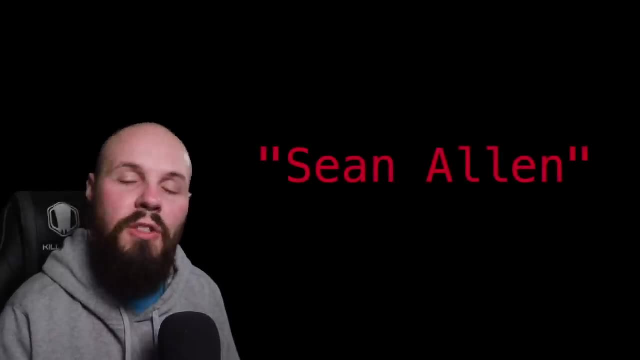 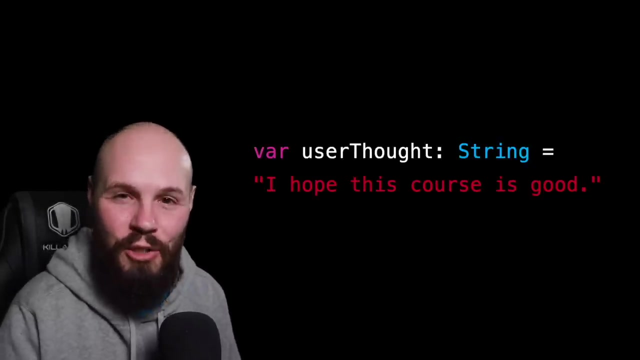 declaring a string, you put it in quotation marks, like you see here. Let's look at an example. We'll create a variable called user's thoughts and that is going to equal. I hope this course is good, right. So that is a string. Another example could be: you know, my name equals Sean, as you see. 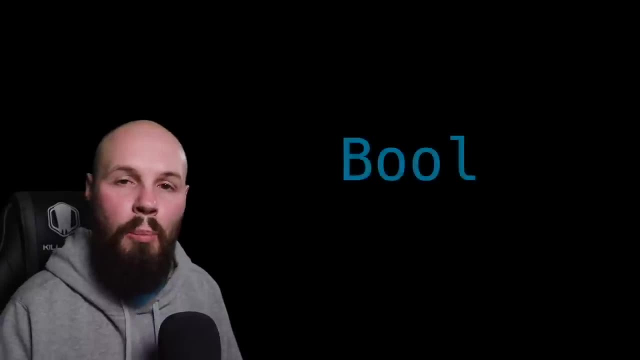 here. So that is of type string. And finally we have our bool type, which is short for Boolean, and that is just true or false. In the example here you can see, we have our variable, which is dark mode on, and that equals true. I know I ran through these quickly, but this is. 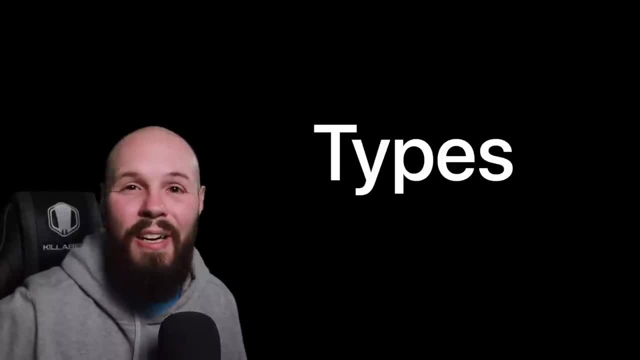 the foundational knowledge that we're going to use and explain throughout the entire course. So you're going to have plenty of time to reinforce this knowledge, But I want to leave you with two pieces of information before we leave the video on types, And that is that. like I said, there are 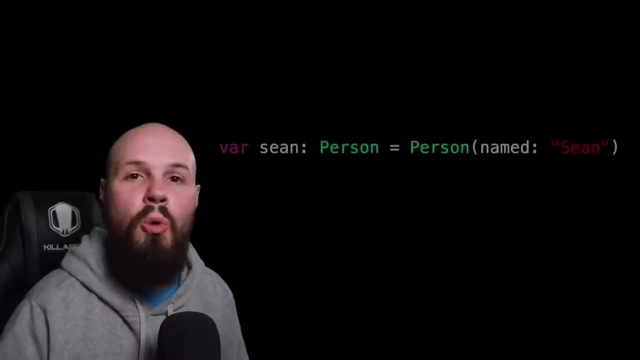 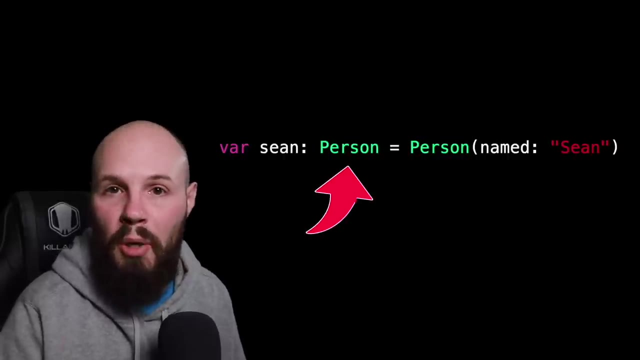 tons of different types throughout Swift And often we even create our own types when we create classes. So let's say, we create a class that is a person- right, You can see, Sean is of type person- and then you create that person. 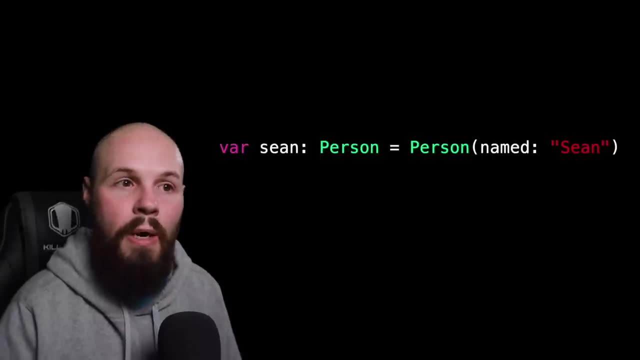 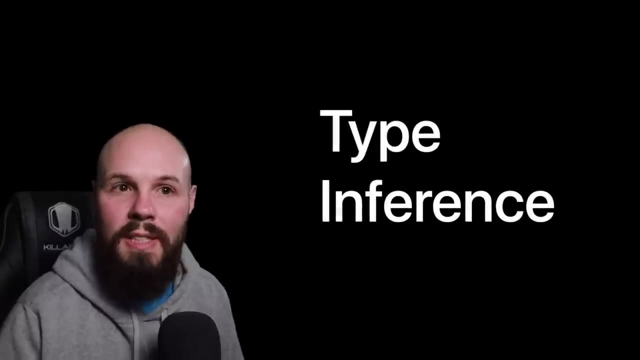 You can create a class that is an object. More on that later in the course, but that's just an example of how it doesn't always have to be an int, a Boolean right. You can create your own custom types. And then, lastly, a big feature of Swift is type inference right. So back to our high score. 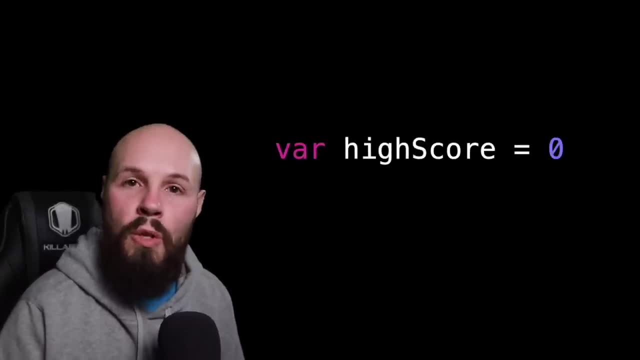 example, if I do var, high score equals zero. Swift is smart enough to know that, because I put a zero there- not 0.76, or 1.89,, it's a zero. Swift is smart enough to infer that. okay, this is an int. or. 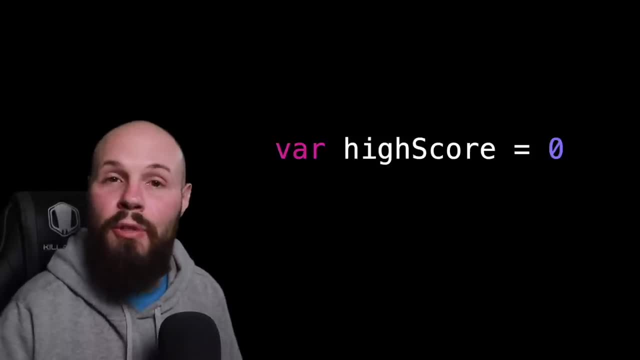 an integer And I would say 95% of the time type inference will work perfectly fine. There's a small subset of time where you will have to manually declare your type, But again, type inference works most of the time. So in future lessons or videos, if you don't see me like, declare the type after my. 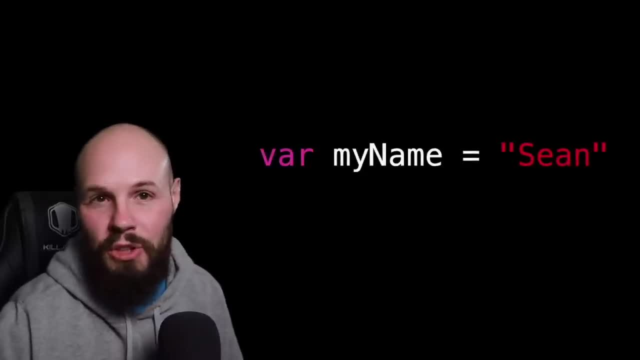 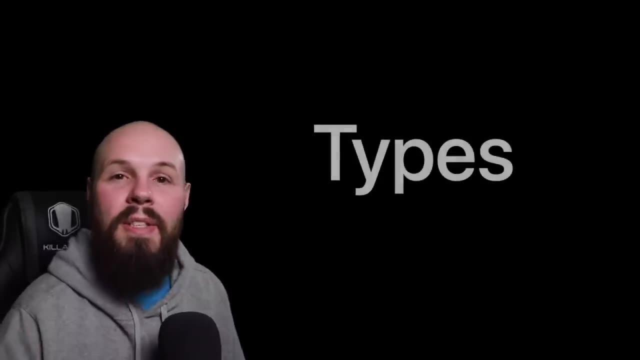 variable, like again var. my name is of type string equals Sean. if I just remove the is of type string. that's type inference at work. So hopefully that avoids confusion. But again, that's the basic knowledge of types. We're going to use this all throughout the course. So if you're interested in, 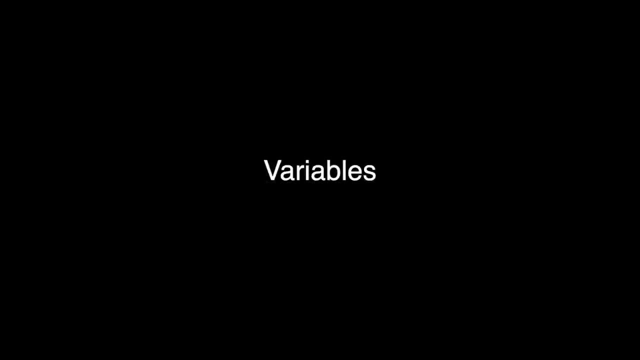 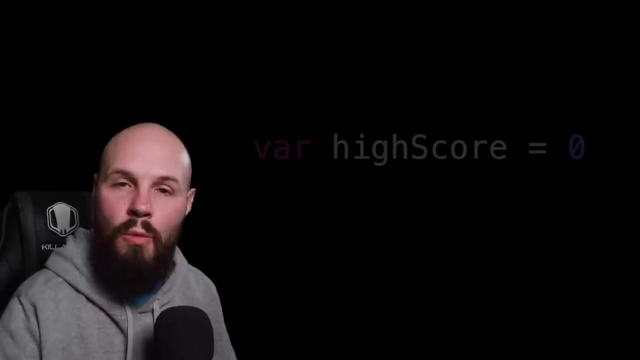 this course so you'll have plenty of practice with it. Variables and constants. we got a little bit of a sneak peek in this in the previous video, when I was showing you how to use types and I was declaring variables, So you may have a little bit of an idea. 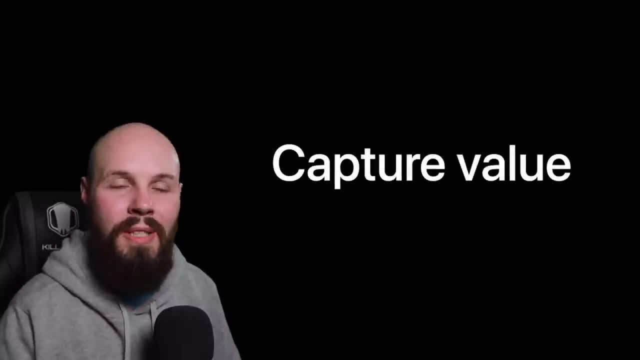 But let's dive into that a little further. What variables and constants do is they capture a value so you can use that value throughout your code base. Right back to the previous example talking about integers, when we said var high score of type int equals zero. 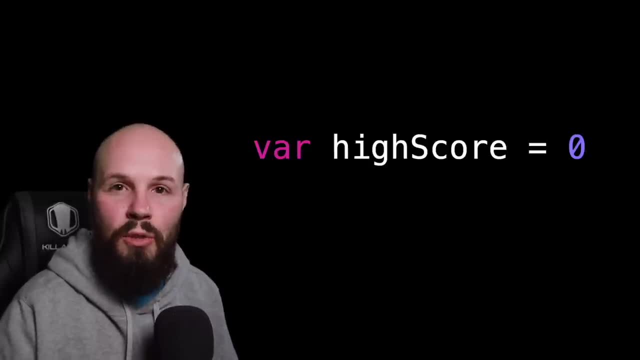 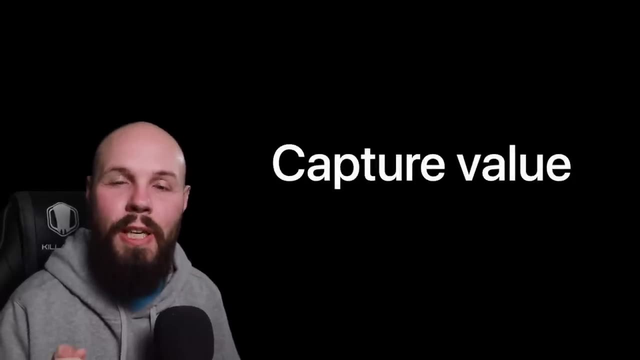 We're capturing the value of zero And now it's in a variable called high score. Now we can use high score throughout our code base. So again, the fundamental knowledge is: variables and constants capture a value. Now what's the difference between a variable and a constant? 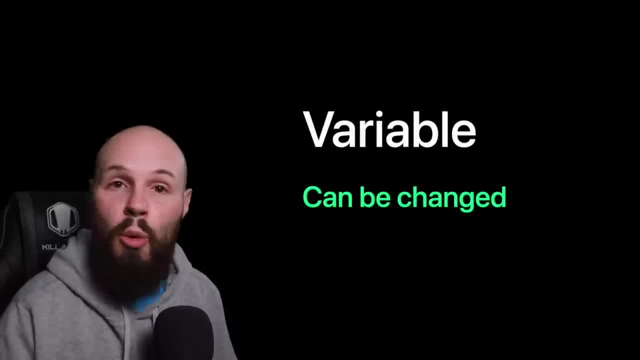 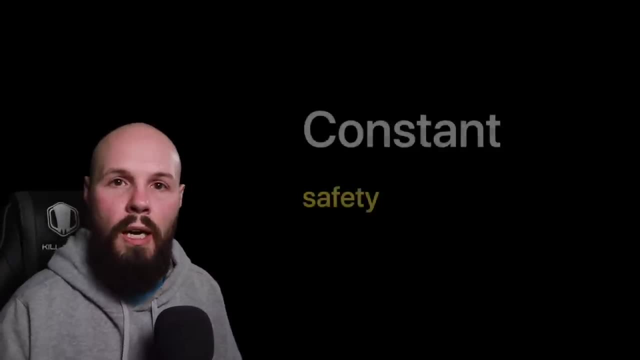 Well, a variable has the ability to be mutated or changed, whereas a constant cannot be mutated or changed, And there's some pros and cons to both right. So if you make something a constant, it's a little bit of a safety feature to where you can't accidentally change it when you don't mean to. 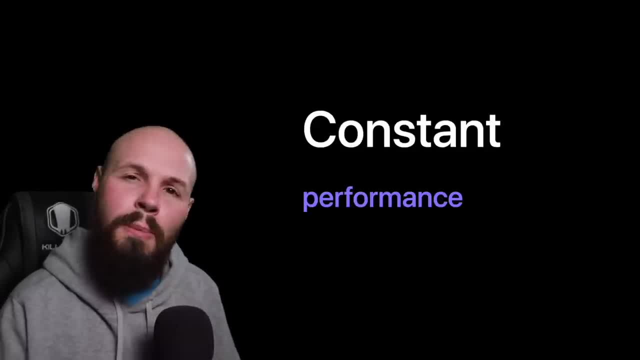 Xcode will yell at you. And then also there's a little bit of a performance optimization, because Xcode, if something can be changed, you know it has to a lot for that possibility, whereas with a constant you say no, this is the value. 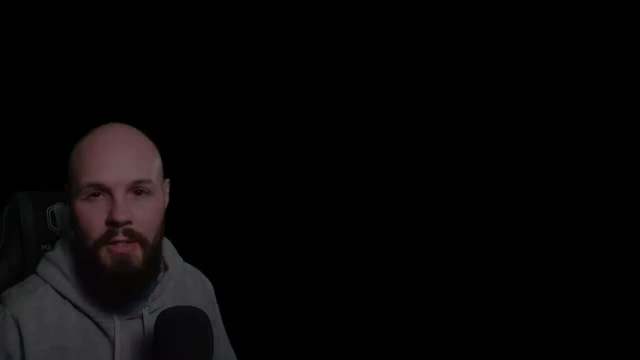 It is not changing. Xcode can optimize that and your code can run faster. Now, in this first lesson, I'm going to show you how to open up a playground and set everything up, But on future lessons we're just going to skip this step. 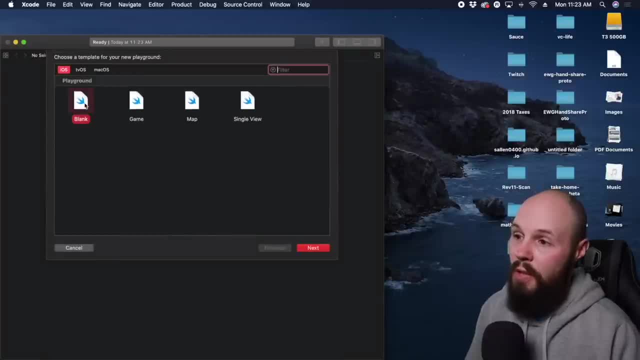 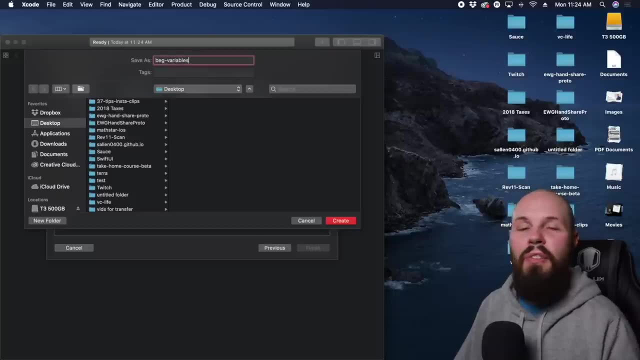 So here, get started with a playground. Click on that, We'll start with a blank one. So hit next. It's bag, dash variables, And I'm prefixing all my stuff with bag because that's how I'm organizing my files all around the beginner course. 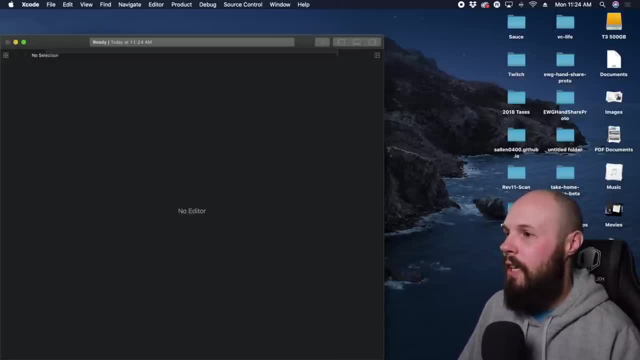 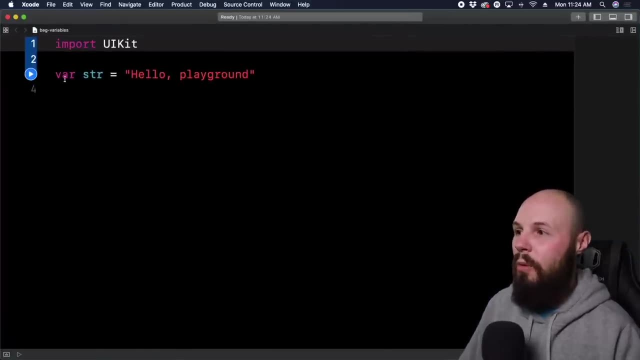 You can name it whatever you like, And I'm saving that to my desktop for now. And let's make Xcode fill up the whole screen for you. There we go, And your playgrounds will automatically start with a variable. It says: hello playground. That's a string. 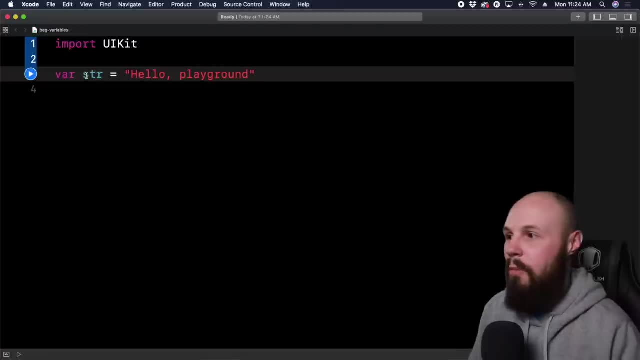 Remember we talked about this in the previous video Like, so just a real quick example. This is a vario called STR. that is type inference to be type string. Because Xcode knows this is a string, All your playgrounds automatically start with that. 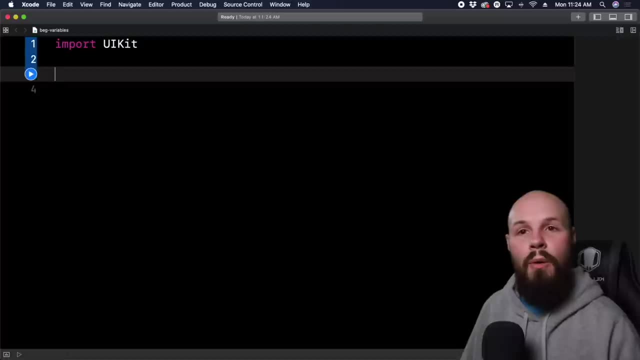 Let's delete this. Don't get ahead of me. Xcode, All right. So let's talk about variables versus constants. Let's continue with that high score example. So var high score equals zero, And again, type inference on the end. I don't have to say it. 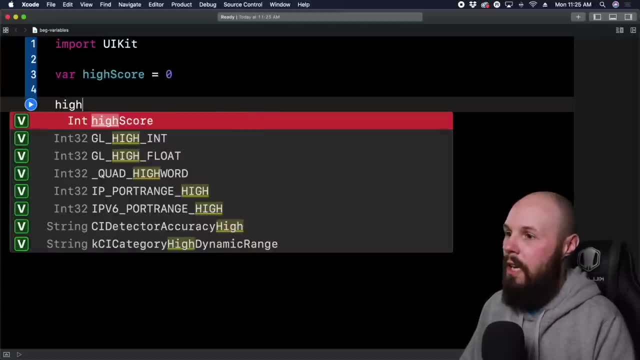 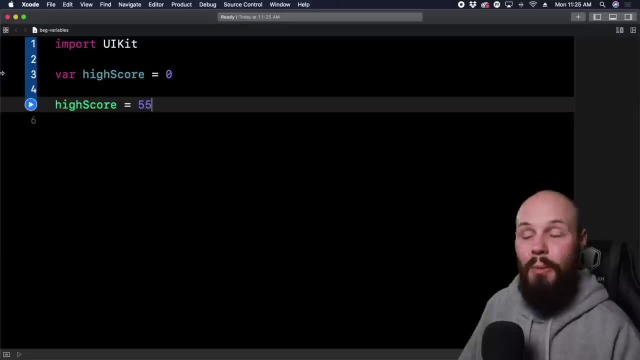 So now I can actually change high score. So I can say high score equals 55. Right, I can update my high score. I did really good on the game, Updated my high score. The reason I can change that is because we declared it with a var, So it's a variable. 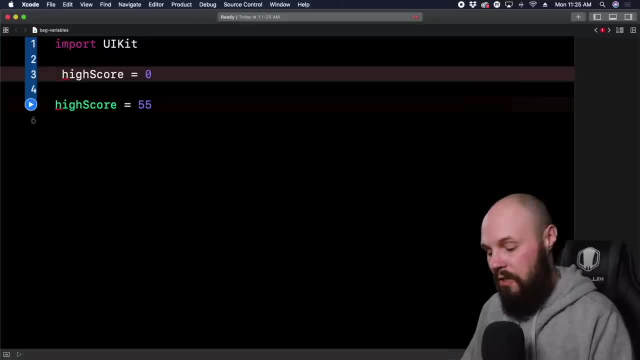 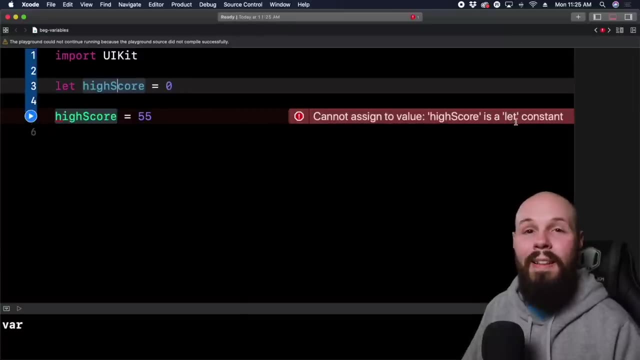 Now if I made this a let, which is a constant. So if you want to declare a constant instead of var, you do let. Now, if I run it, you'll see it's going to say: cannot assign to value high score is a let constant. 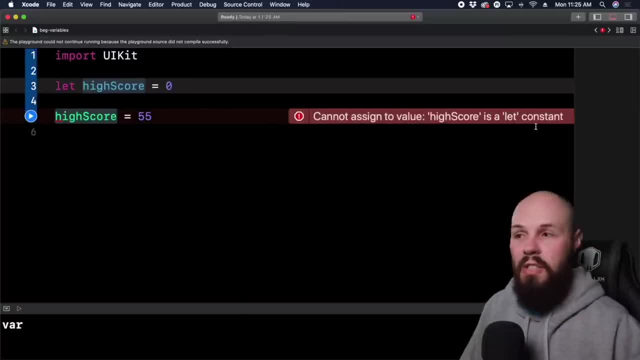 So, like I said, if it's a let, Xcode will say: no, you can't change this. If it's a var, you can change it, And real quick, just to avoid any potential confusion when developers are discussing code. 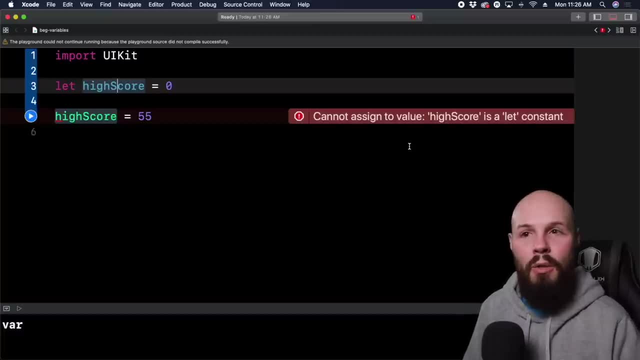 and you may hear me say this throughout the course is: oftentimes they'll just call these all variables. whether it's a let or a var, You may not distinguish between the two right. Oftentimes you just say: create a variable for that and do this with it. 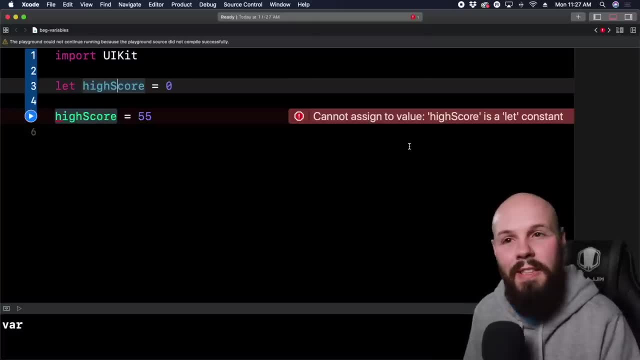 And that's because when discussing code you may not know all the specific implementation details if it needs to be a let or a var. So if I say, hey, we're going to declare a variable here, I'm not always saying it has to be var, right. 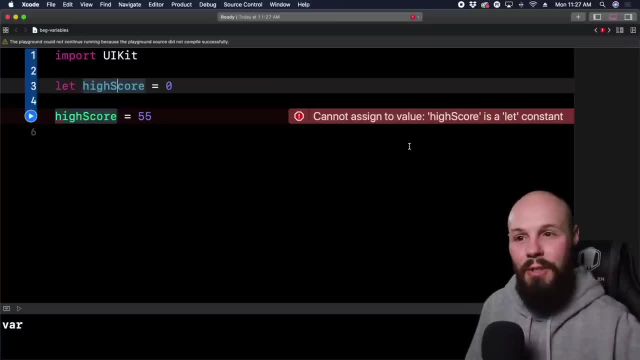 It could be let, So variable is kind of like the overarching way to refer to it. And then deeper, you know the difference between let and var depends on your implementation details. So again, to avoid any future confusion if I call something a variable, 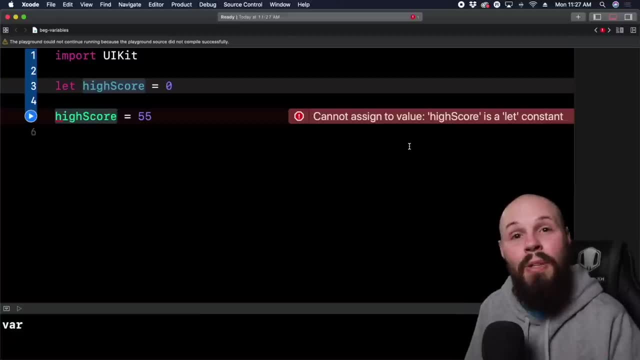 but I make it a let. that's why. But again, the textbook answer right So somebody could come up and correct you because technically they would be correct. You should call it a constant or a variable. But again, oftentimes in just common conversation, 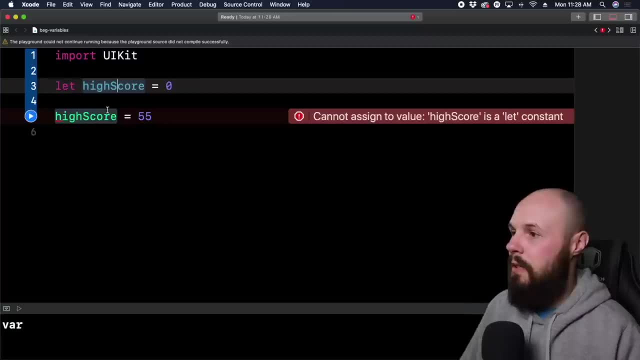 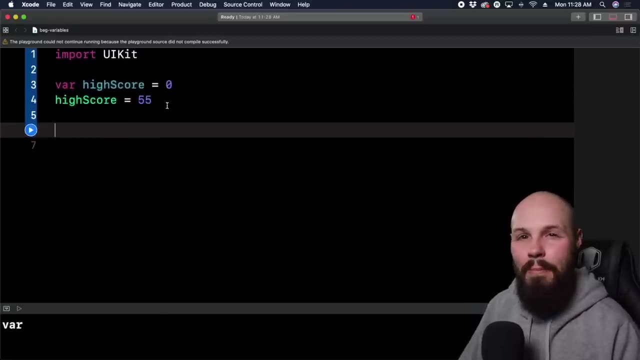 we just call them variables, So hopefully that avoids future confusion. All right, let's change this back to var And let's give two more examples to just really really drive this point home. So something like a name of a person, right? 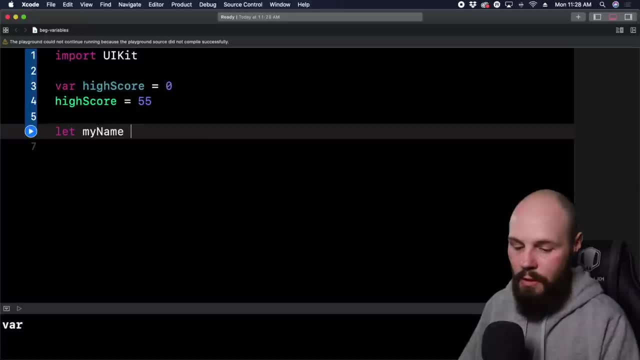 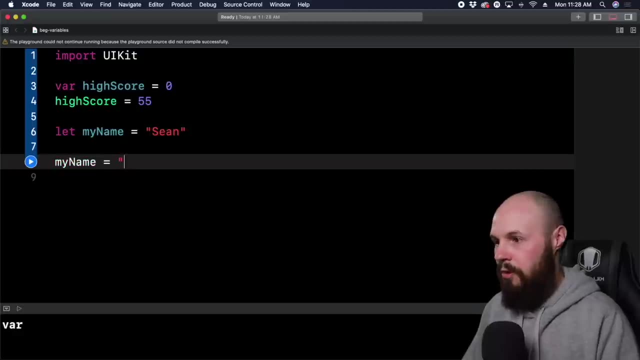 You don't want to change that, So you would do something like: let my name equals and this is- this is a string here- Sean. So now I can't just do my name equals, you know, Joe, right, It'll yell at me, right? 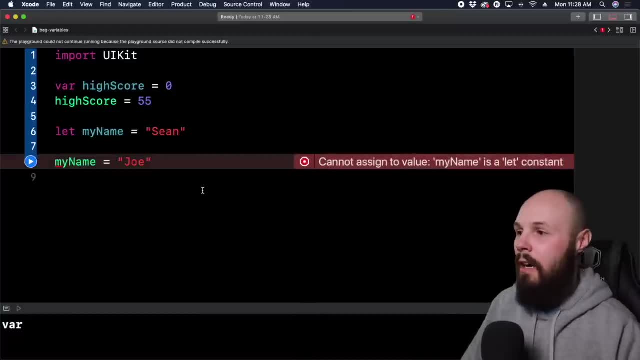 Because my name is a let Cannot assign value of my name. It is a let constant, But something. let's delete this More along the lines of: you know var current active users, right, That's something that is always fluctuating. 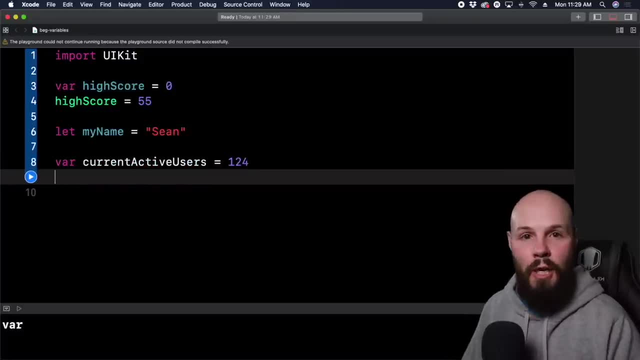 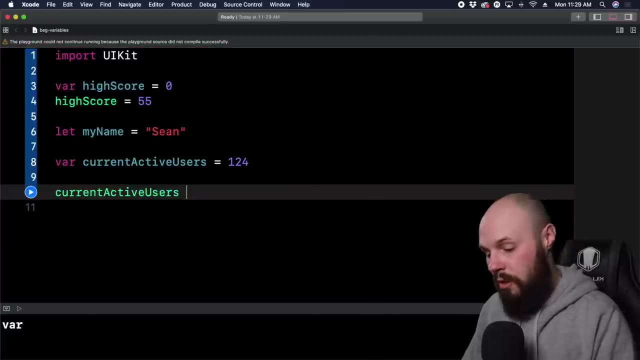 We'll say that equals 124.. Now I can change and update that right. Like, say, I get a huge spike in traffic on my app. I can, you know, I can change that. You know. say, okay, we need to set current active users equal to 1,458, right. 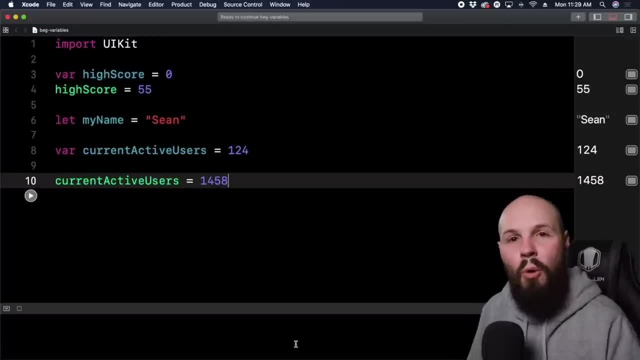 And that can be changed because that is a var, And to reinforce the core concept of variables and constants. they capture a value, So you can use that value, For example, this current active users value. I can use that throughout my, my code base. 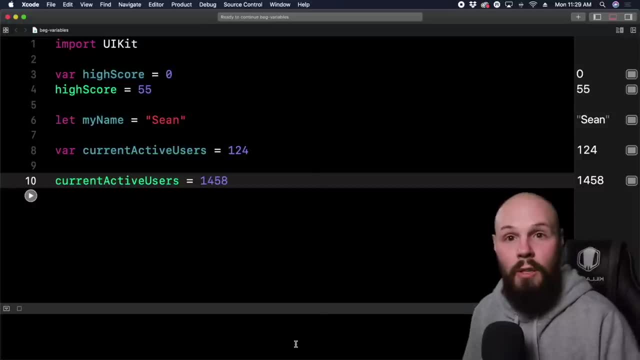 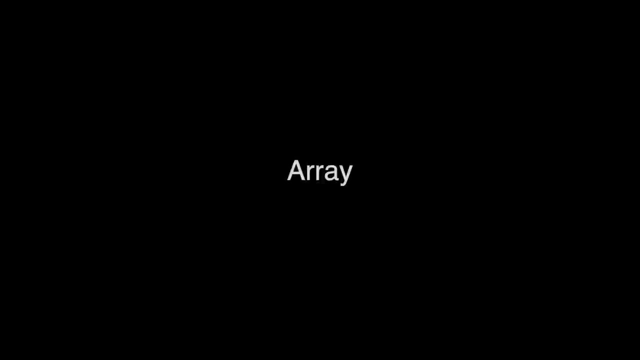 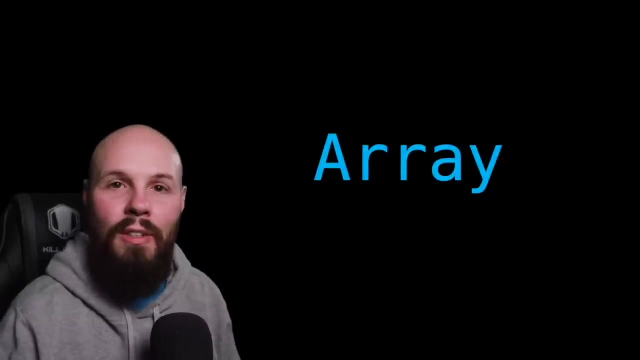 For example, you know, if current active users is less than four, print out traffic is way down, right, I can do stuff like that based on the value that's captured in this variable. Now let's talk about arrays, and array is a container or a list of objects. here on the screen is a visual aid to hopefully help you understand the concept of an array. 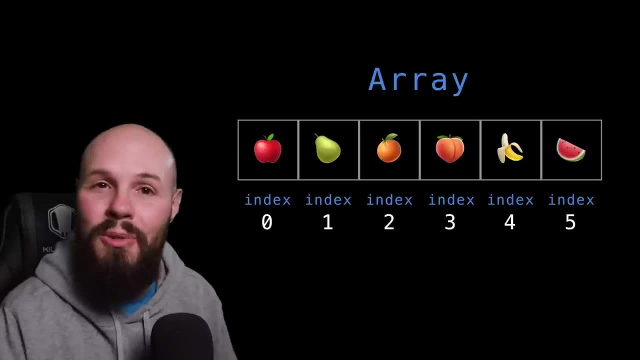 For example, this would be an array called fruits. As you can see, there's various different fruits in this list. Now, one key thing to know about arrays is that this list is numbered But, as you noticed, it's zero indexed. 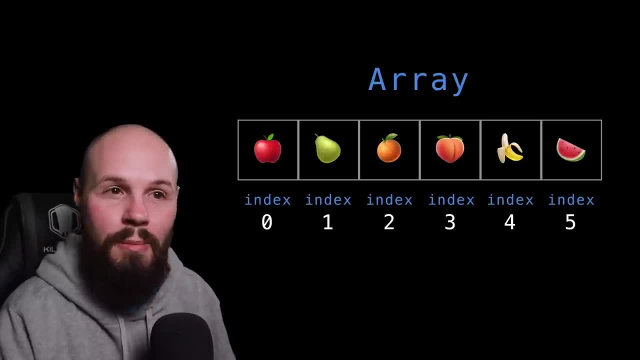 What that means is the count starts at zero. So the first item is not one, It's zero, right As you can see, zero One, two, three, four, five. not one: two, three, four, five. real quick, take a second to let that sink in, because I guarantee you you're going to have an error, because you forgot this at some point early in your career. 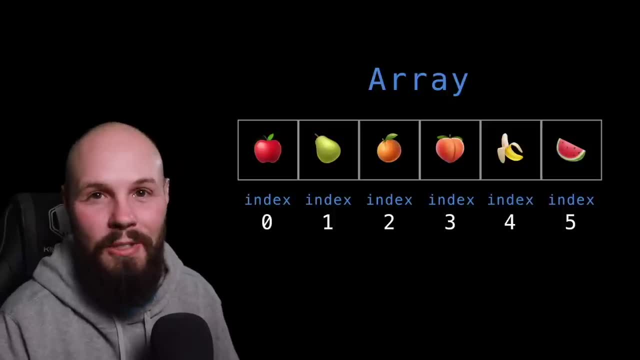 So this is very, very important. It's a fundamental thing to know about arrays. Now, of course, arrays don't always have to be fruit, right, We can have an array of integers, right, Let's say we want to call this ages. 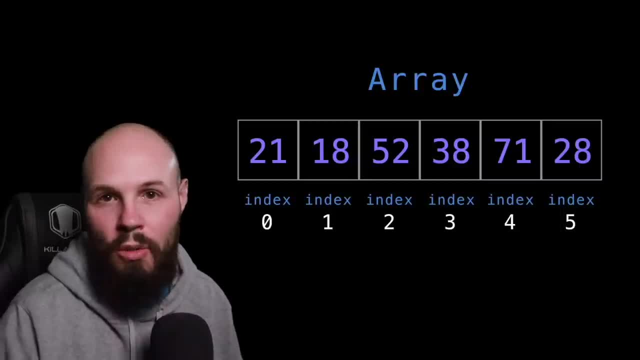 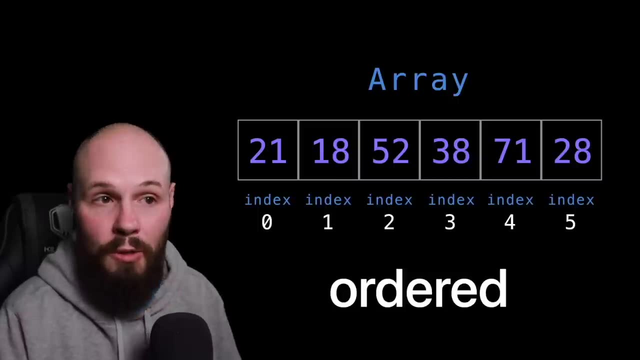 And this represents the age of everybody currently taking this course. Another thing to know about arrays is that they're always in order. Now, by in order, I don't mean alphabetical, I don't mean numerical, As you can see, with these different ages, right. 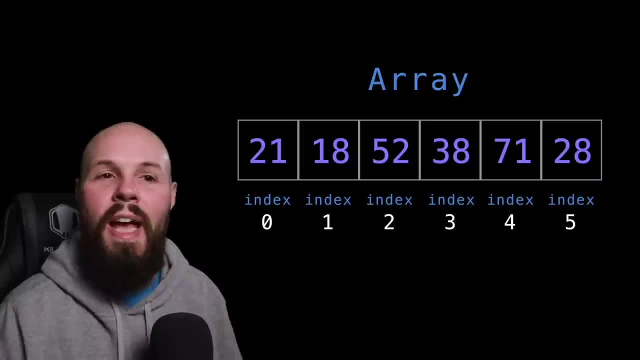 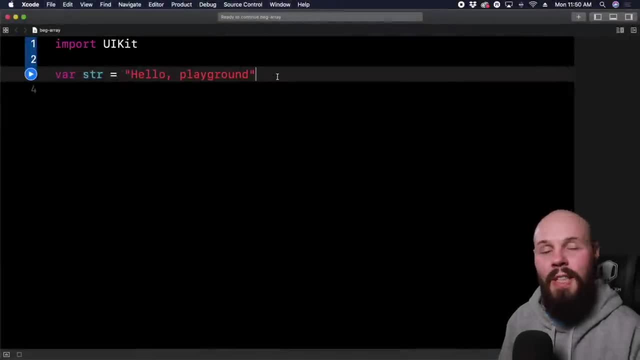 I mean the order that they were put into the array. Let's illustrate that and a lot of other things you can do with an array in some code. Here I am in a brand new playground. Remember last video I said I wasn't going to go through the step every time of like file new playground and naming it. 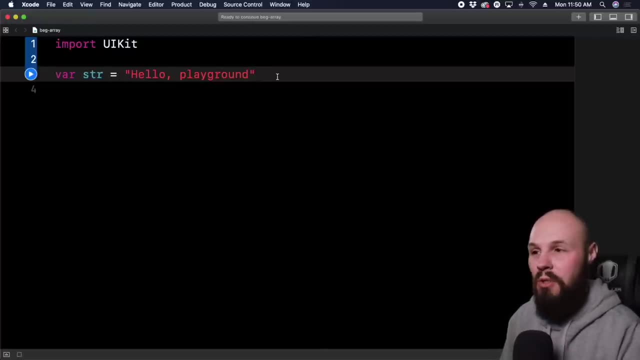 So go ahead and do that on your own and you'll see this empty playground to start with. All right, so let's create that array, So var ages equals and it's an array of, let's say, the different ages: 21 comma space, 55 comma, 19.. 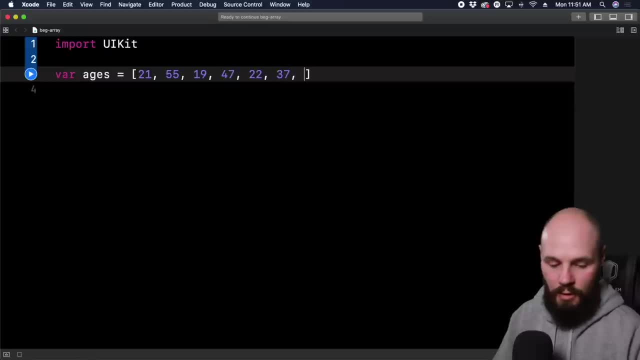 I'm just going to put in like eight of these Real quick, just random numbers and whatever: 71. That's it. I think there's what Eight of these in here? Cool, Now, real quick, we just declared this array. 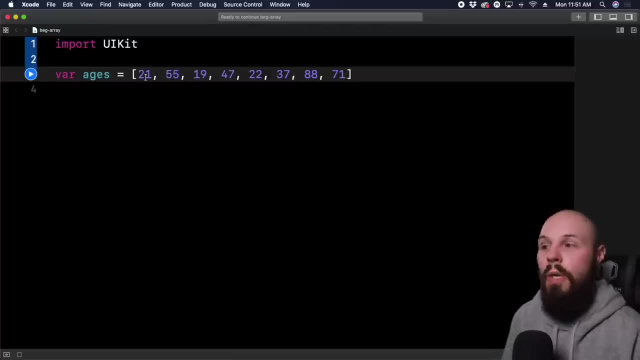 And what I talked about was the order that I put them in. So you know, I put in 21 first, then 55, then 19.. That's what I meant: that they will always be in order. Again, not numerical order. 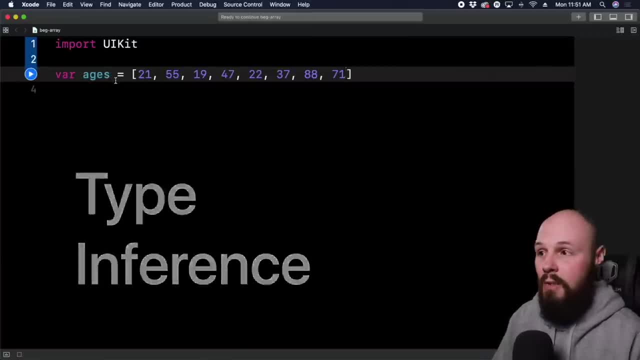 And again back to type. inference. Ages knows that it is an array of ints, because I've put all ints in here. Now, however, let's cut these. I'm going to do command X to get rid of them, because I'm going to paste them back in. 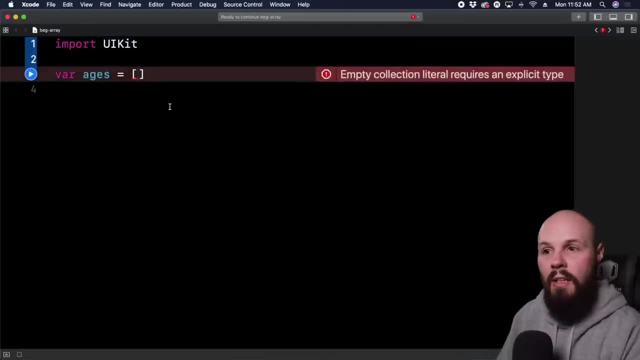 So I'm going to type them Again. now I have an empty array But you'll see Xcode is saying empty collection- literal requires an explicit type. When I had all integers in there, Xcode knew all right ages is an array of ints. 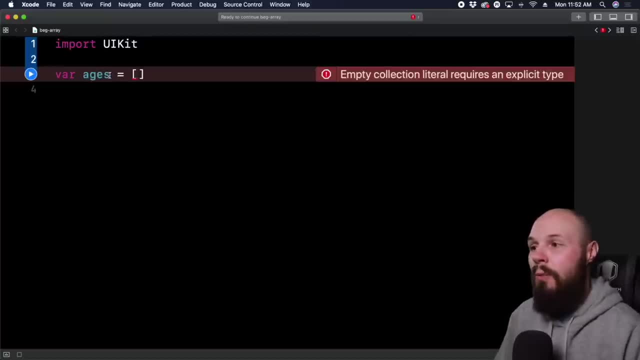 But I don't have anything in there, so it doesn't know. When you want an empty array- which is actually quite common- very often you'll declare an empty array, But if you do that, you have to give it a type. 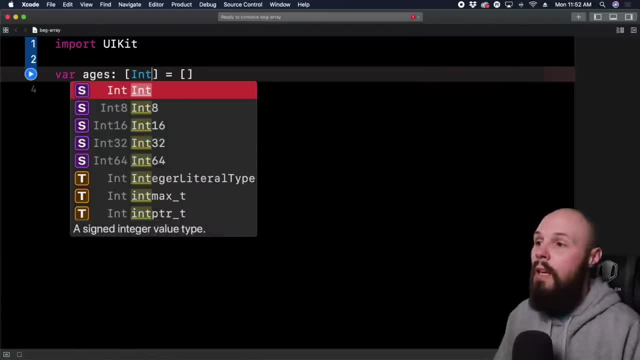 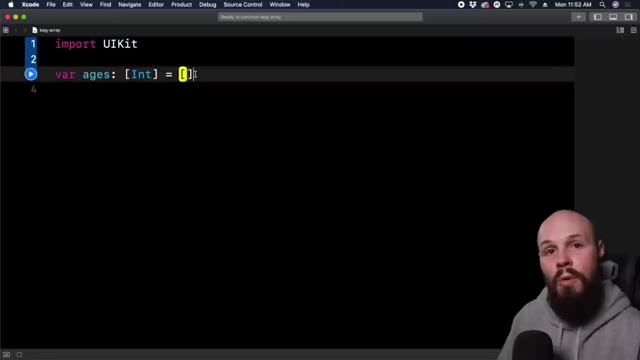 And you have to put the type in the brackets to let it know it's an array. So this is saying ages is an array of type ints. So that way, even if you declare an empty array, Xcode knows: hey, I'm expecting an array of ints. 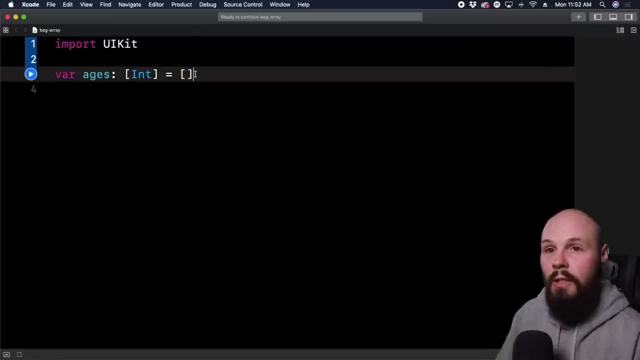 And then later on, if you try to put in a string or a boolean, Xcode's going to be like: no, no, can't do that. This is an array of ints, But let's put those ages back in there. 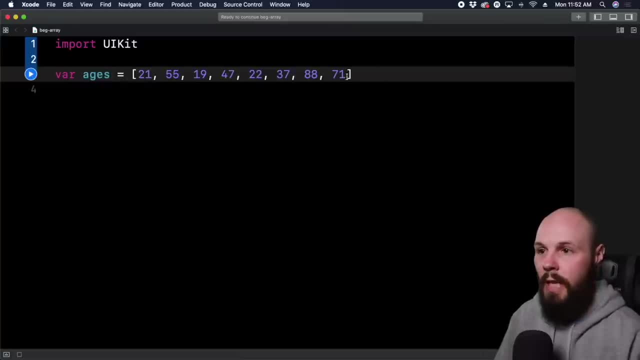 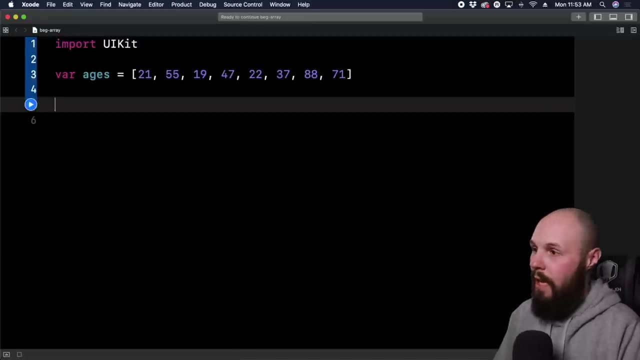 And we can delete our type declaration because we don't need that. We'll use the type inference. Now let's talk about some of the features of an array and how you can use it. So, first up, we can always get the count of an array by doing agescount. 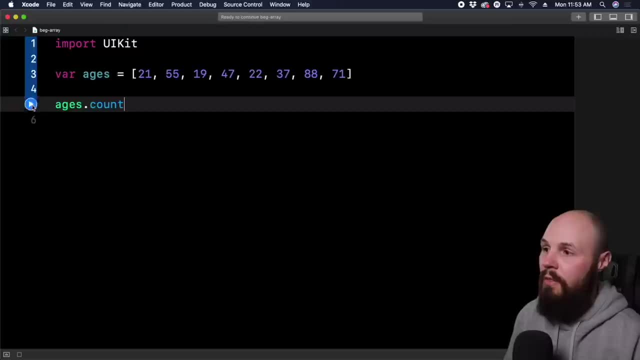 And this gives you the number of items in the array. So if I hit this little play button on the left to run it, you'll see on the right we printed out eight. So that means there's eight items in this array And you can count it for yourself. 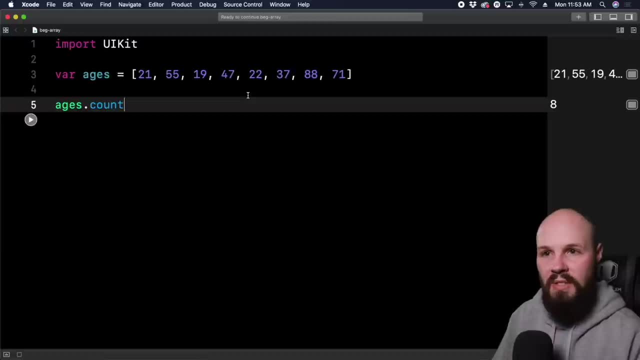 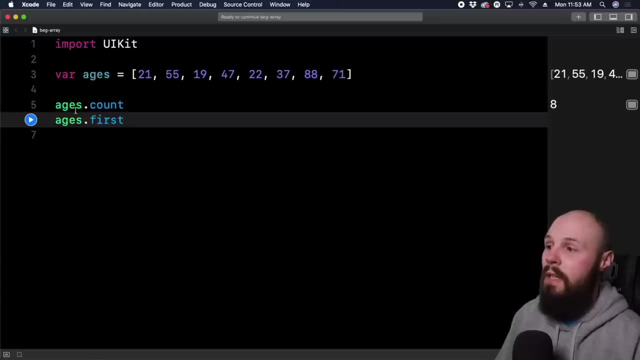 There are, in fact, eight ages in there. Another common thing you want to do with arrays is access the elements that are in there. For example, you can do agesfirst And this will return the first item in this array 21.. 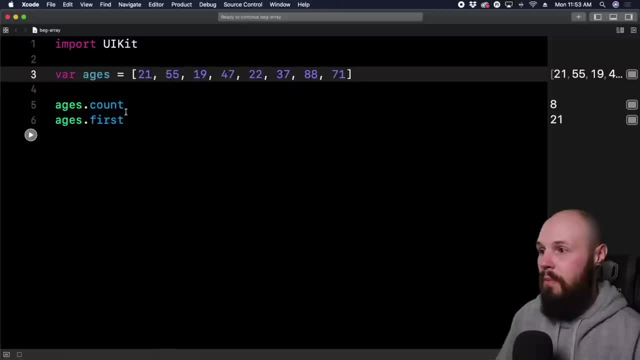 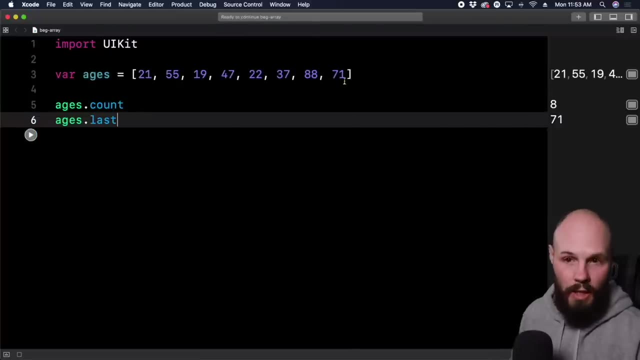 You can see it: print out 21 here. 21 is the first age, Same thing. you can do ageslast, Same thing. Now it's going to give me 71, right, As you can see right there, because that is the last element of the array. 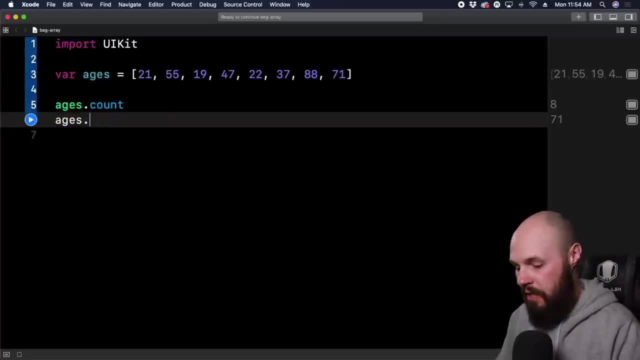 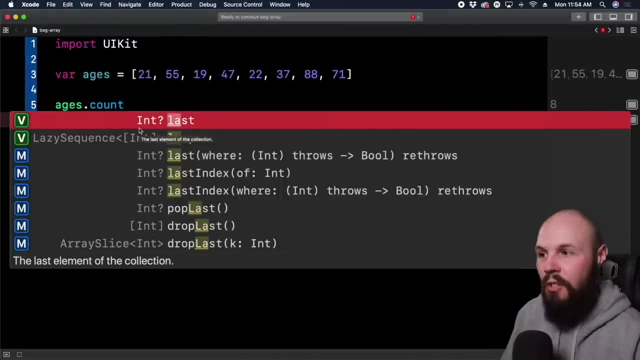 Now, real quick, A little sneak peek into optionals. You'll notice ageslast was an optional. This question mark means it's an optional. We're going to dive into that later. I'm not going to get into that now because we're just starting out. 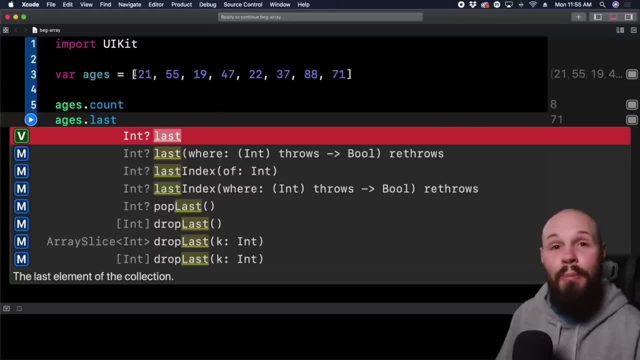 But the reason it returns an optional is because ages could be an empty array, And if you have an empty array, what's the last object in an empty array? Like nothing, So you don't want the app to crash. So that means it returns an optional, which means it can be nil. 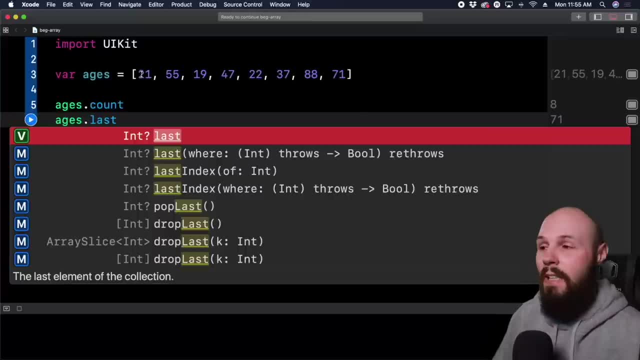 Again, if that was confusing. you don't know what I'm talking about. We're going to discuss that in a later video, But I wanted to explain to you what this little question mark meant. That basically meant that this can be nil. 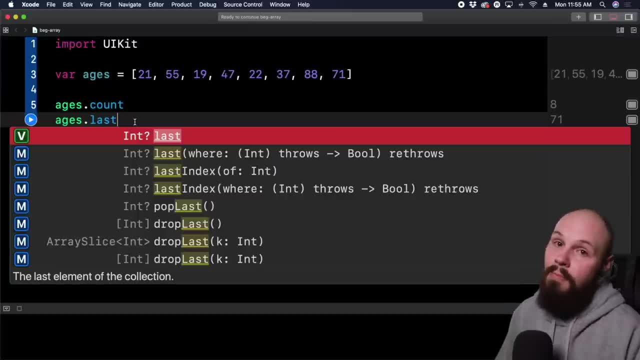 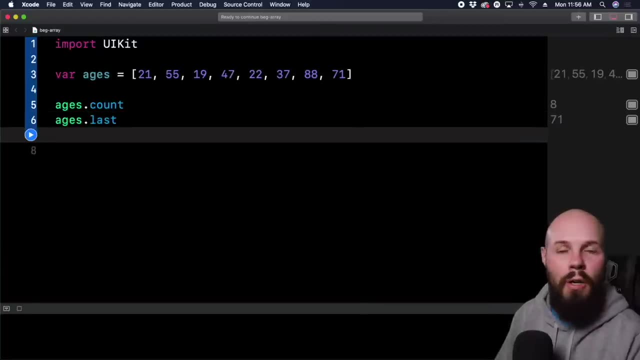 This can have no value. And again, in the case of an empty array, there's no last object in an empty array. All right, more accessing items in the array. So we did first, we did last. What, if you want one in between? 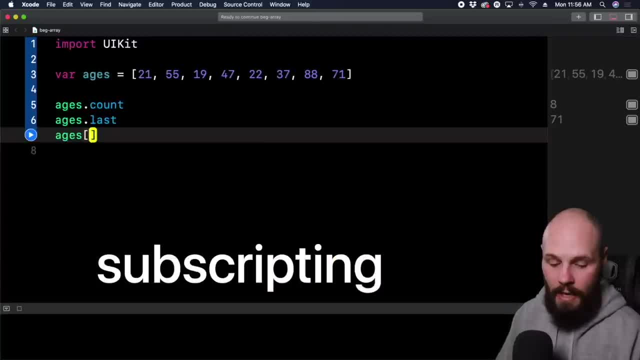 Well, you can do ages, and this is called subscripting. We do brackets and then put in a zero. This is where you put in the index number. So ages at index zero is going to be 21.. So it's going to be the same as first, because we did index zero. 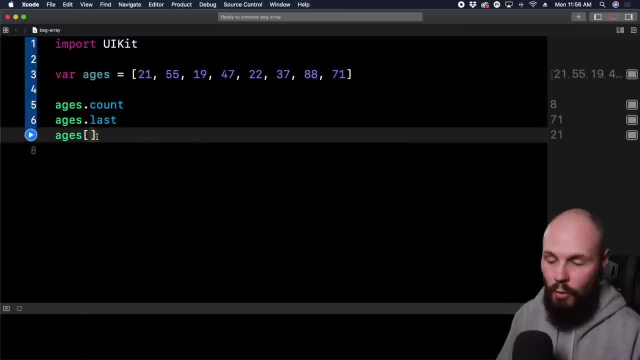 You see it prints off 21 there. But you can also do the fourth one You want for three. Remember: zero indexed. So the fourth item is going to be three, because it goes zero, one, two, three. So now the fourth item is 47.. 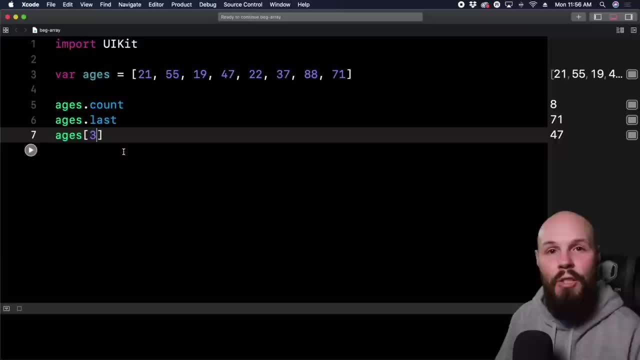 See it prints off 47. So that is how you can access individual elements in the array. And again this goes back to the array being ordered. It's always going to be in the order you put it. in. That way you can reliably say: give me the item at index three. 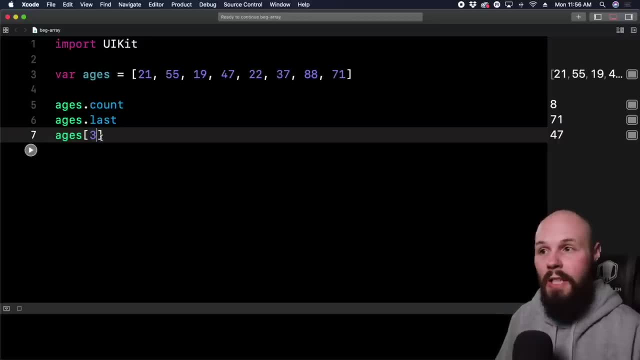 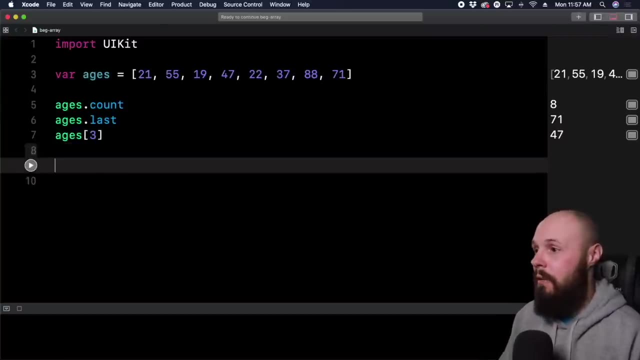 and it's always going to be the same. If it was not ordered item at index three, it would be different every time. So that is why the array is ordered. Now, aside from accessing items, we can actually manipulate our array. Let's say we got a new student and we wanted to add a new age to the end of it. 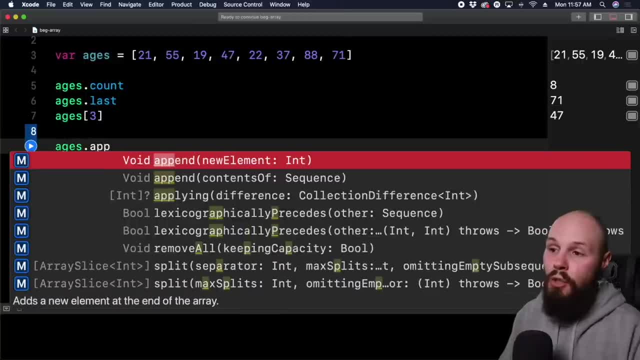 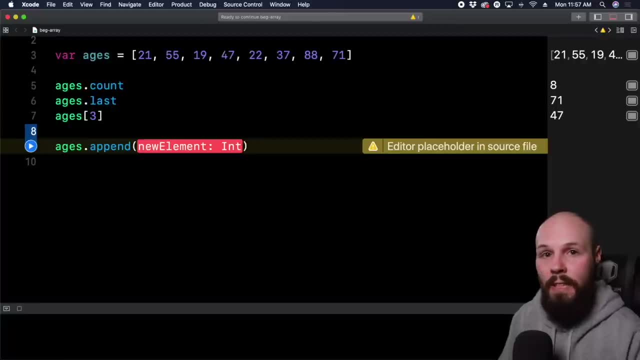 So I can do agesappend and you can see new element int. And this is type safety in action. right, Because ages is an array of ints, it's not going to let me put anything other than an int in there Again. this is the whole safety aspect of the Swift language. 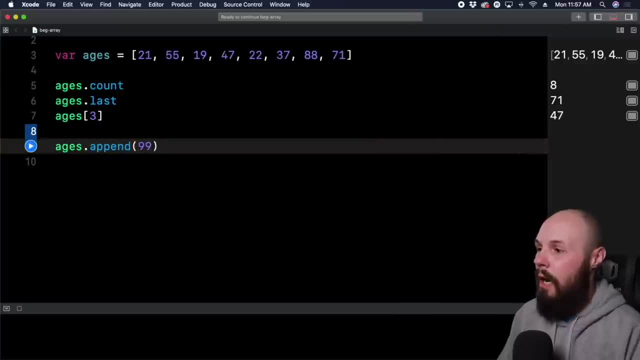 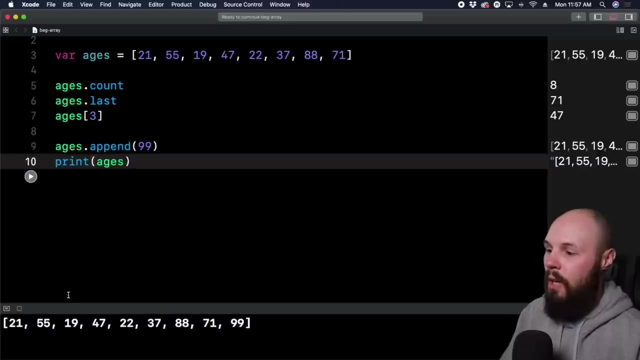 So let's say we want to put 99 in there for our new student. Now a way to print out stuff is do print ages, And if I run it down here in the console at the bottom, it's going to print out my ages. 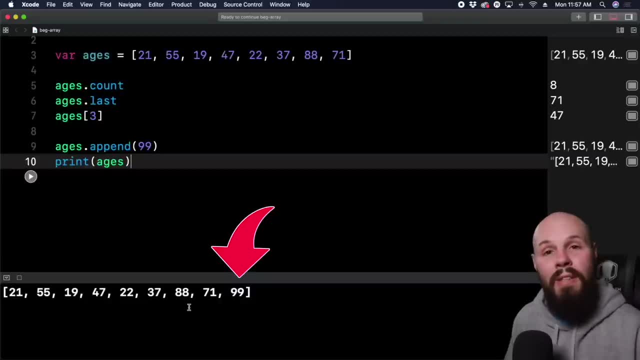 And now you can see 99 is now appended. So the thing when you append stuff is you're appending it to the end of the array. So that's why 99 went there. And let's say you didn't want to append it to the end. 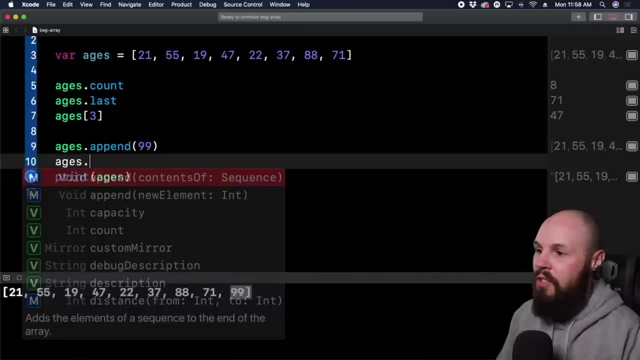 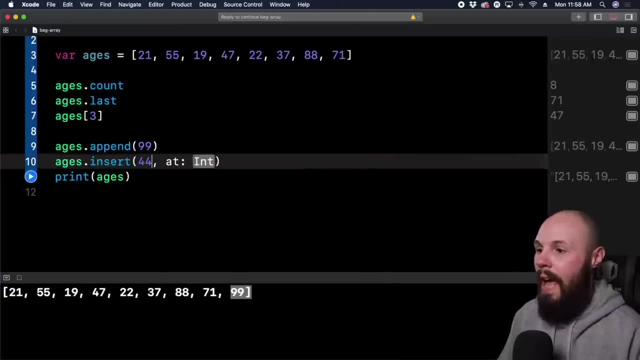 You wanted to put it at a specific spot. You can do agesinsert and you can see new element which is an int Again type safety. So let's say we want to put 44 at and now we're putting an index right. 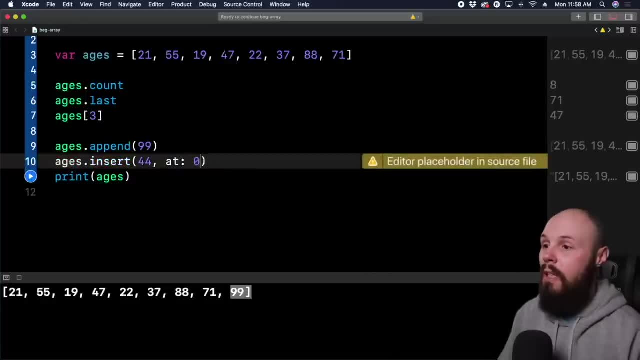 We want to put it at index. let's say zero. We want to put it at the beginning. So insert 44 at index zero, right At the beginning. Now, if I run it, we're going to print ages down here. 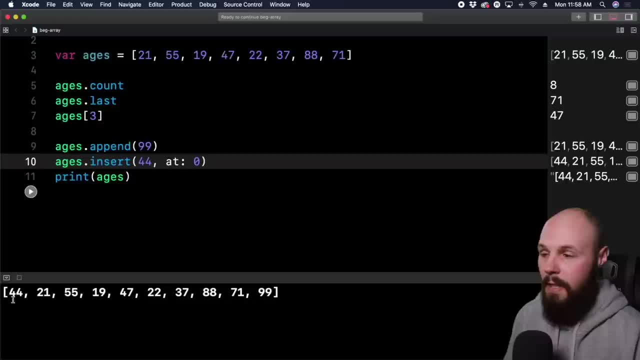 And now you can see 21 is no longer at the beginning, 44 is at the beginning. And the last three things I want to show you is how we can sort our array, how we can reverse our array and how we can shuffle it right. 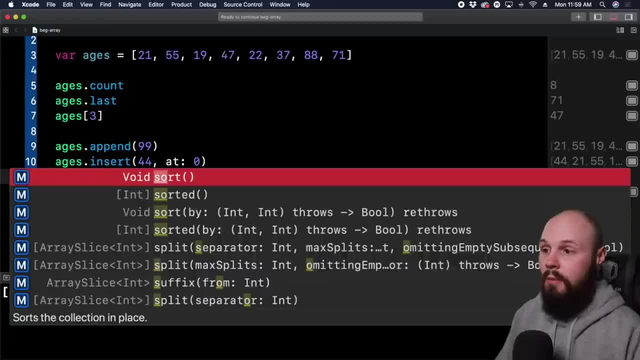 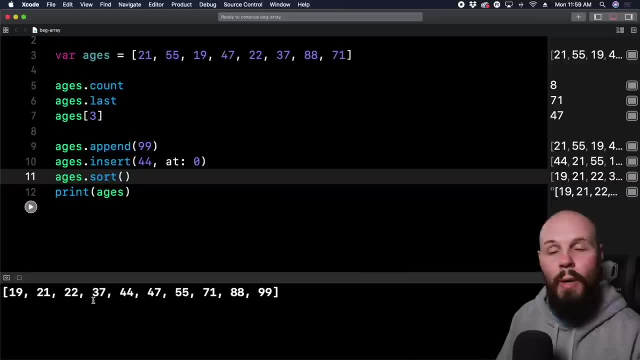 So let's do that. So agessort, and you can see if we print it now. we're going to get this array in numerical order right: 19,, 21,, 22,, 37. So sorting an array is as simple as that. 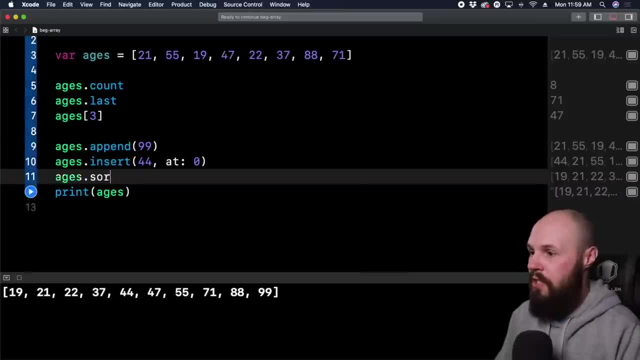 And we can do the same thing to reverse our array. So if we do agessort, reverse, there you go And we run it. Now we didn't do sort anymore, So it's going to reverse what's actually in there on line three. 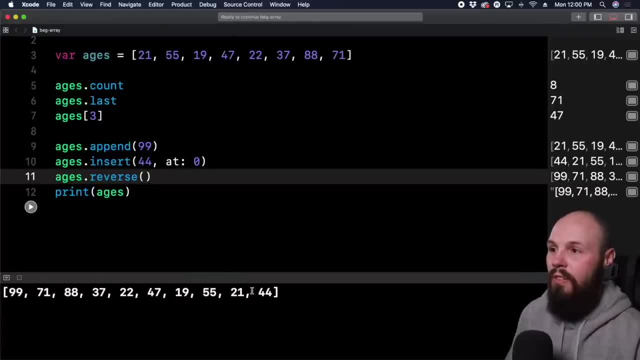 Or actually no, we added the 44. So 44 is, at the end, 21,, 55. You can see it's in reverse order from what we have up here, And then, as you may be following along here, we can do shuffle as well. 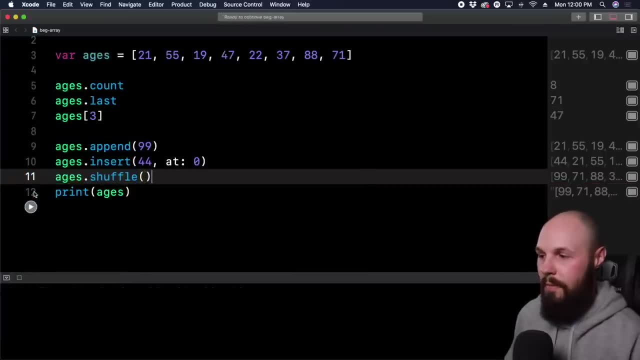 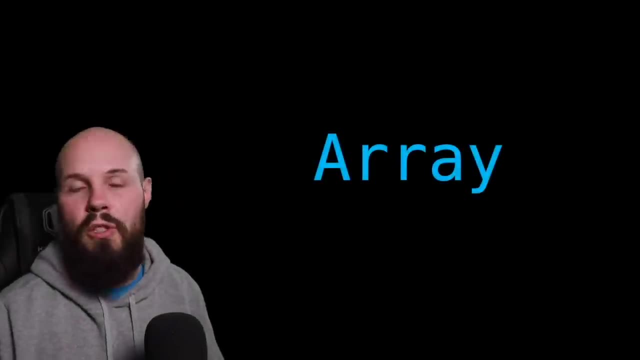 Shuffle And that will shuffle up all the numbers in the array. So you see, we got the array down there and now it's all shuffled. So those are some basic things you can do with an array. Now. arrays are used so much throughout code. 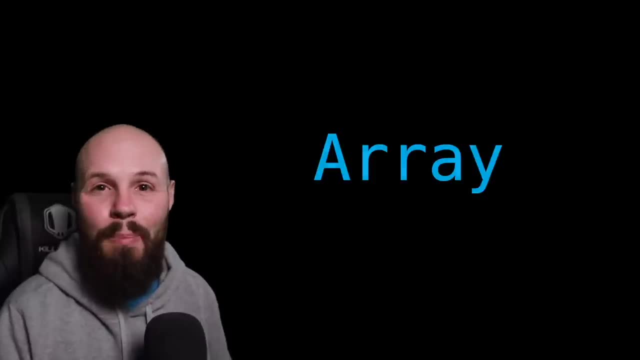 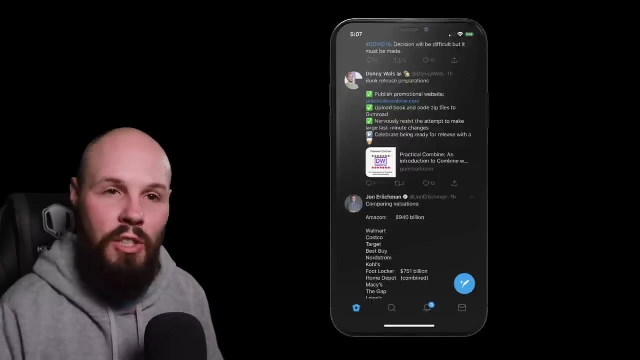 and building apps. A very common thing that you may see on a day-to-day basis is maybe your Twitter feed right. Your Twitter feed that you're scrolling through is an array of tweets. It's just a list of tweets that show up on your screen. 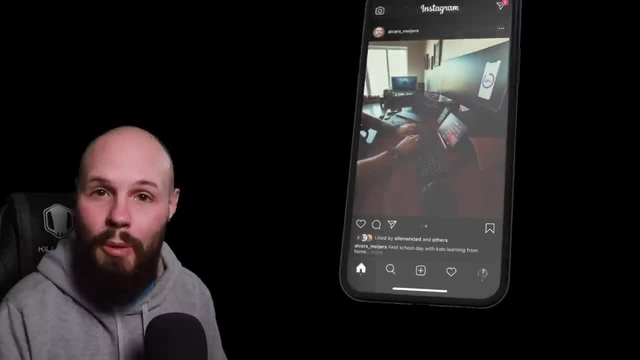 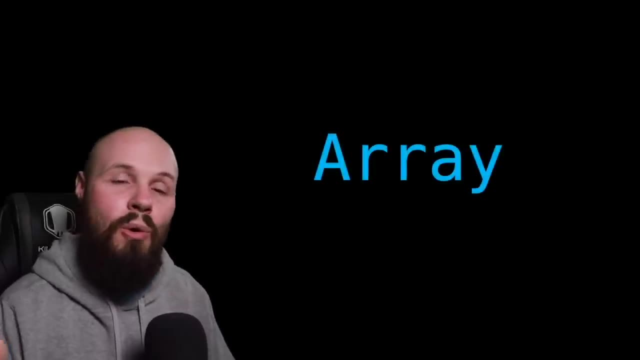 And same thing with your Instagram feed. Your Instagram feed is an array of posts that show up on your screen, So arrays are used everywhere. It's a very foundational knowledge. Hope you got that. As always, ask questions in the comments or on the Slack channel. 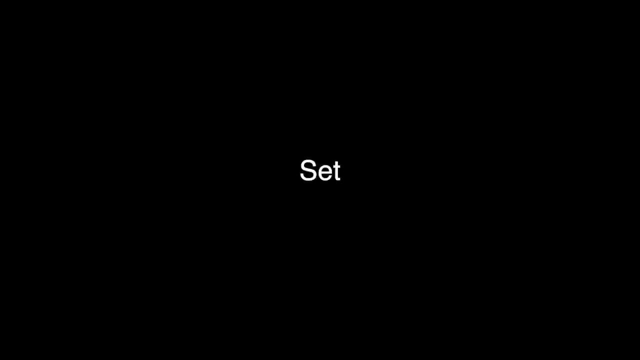 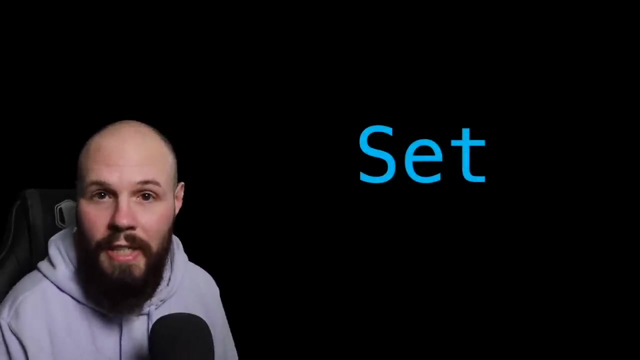 On to the next video. Let's talk about sets. Now. a set is pretty similar to an array in that it is a collection of items. However, there's some key differences between sets and arrays. First up, a set is unordered. 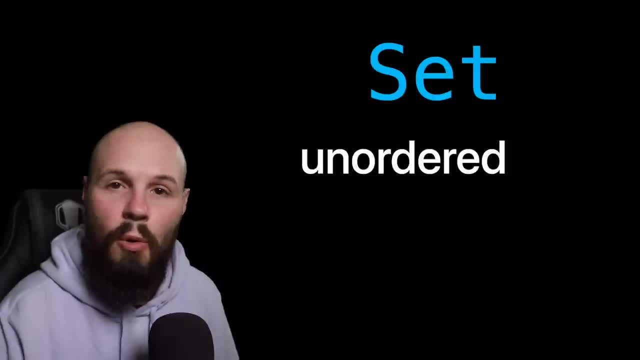 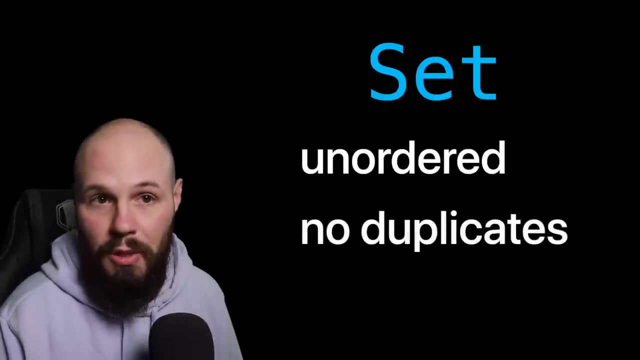 Remember last video? we talked about arrays being ordered and they would always stay in the same order provided you don't change them. Well, a set cannot guarantee any order. Next, a set cannot have duplicate values. If you remember the array that had all of our ages? 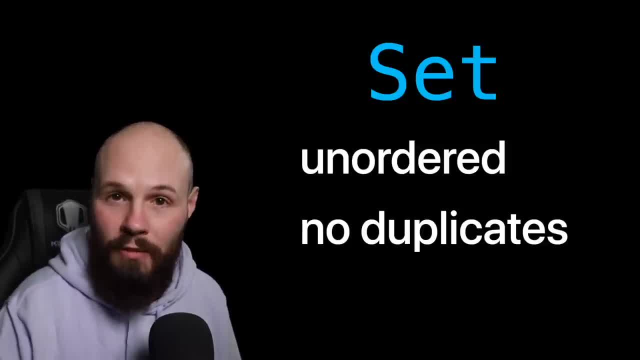 from the students in the course. well, in an array we can have duplicate values in there. However, a set can only have one of those values, no duplicates. So you may be thinking a set is not ordered, I can't have duplicates. 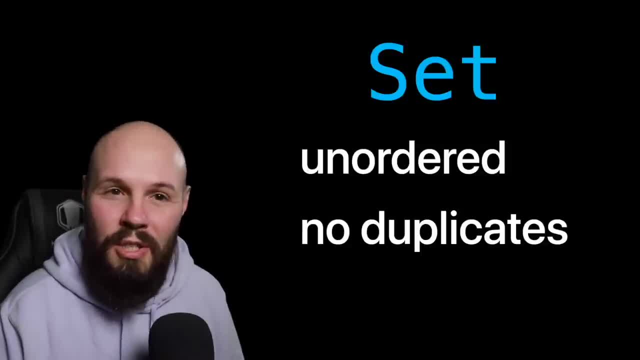 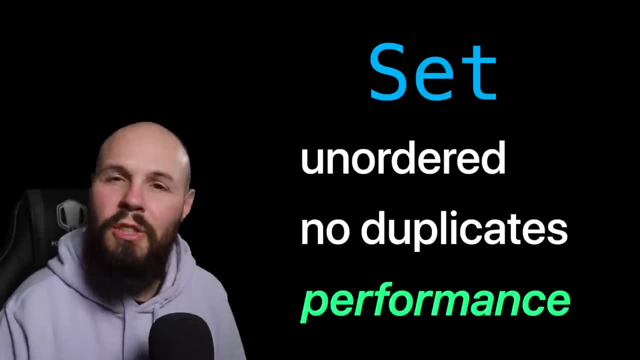 Like: why would I want to use a set? Well, one big advantage to a set over an array is performance and speed. Sets have faster insertion, removal and lookup. And to illustrate all these points, let's dive into some code. 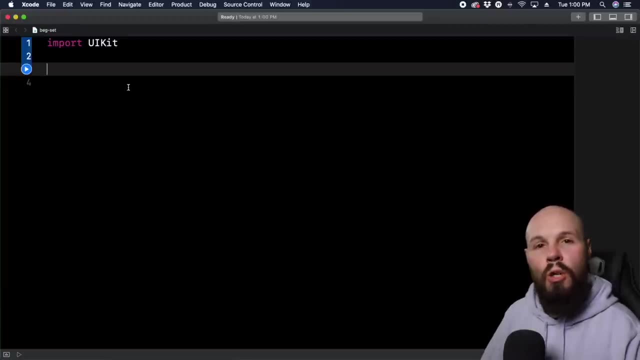 Here I am in an empty playground. Go ahead and create that on your own. To start, we're going to recreate that array, not a set- our array of ages, just to, because we're going to use this as comparison to help really illustrate the differences in a set. 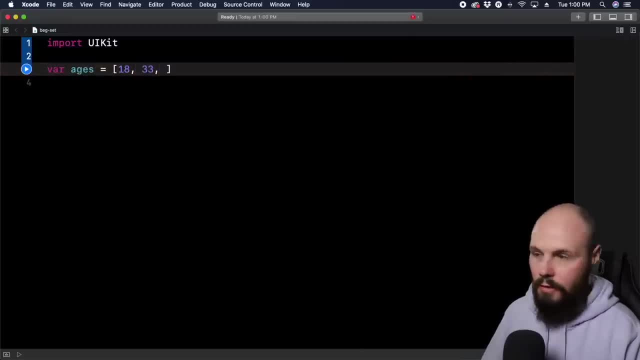 So I'm going to throw in a few random ages in here: 18,, 33,, 55,, 17,, 94,, 20, 26.. Okay, cool, Just some random ages, And actually let's put some duplicates in here. 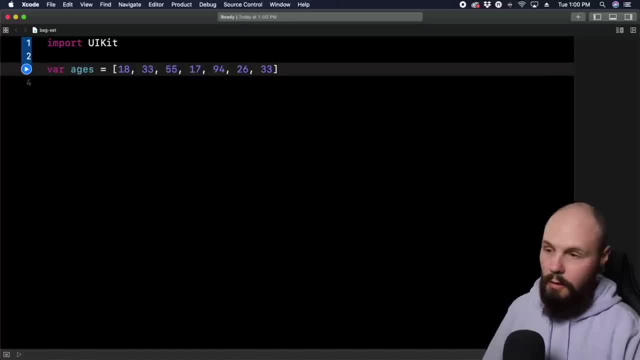 just to illustrate that we can have duplicates: comma space 17,. right, So you see, 17 is a duplicate and 33 is a duplicate. That's fine in ages. So again, we're going to use this array to learn about sets. 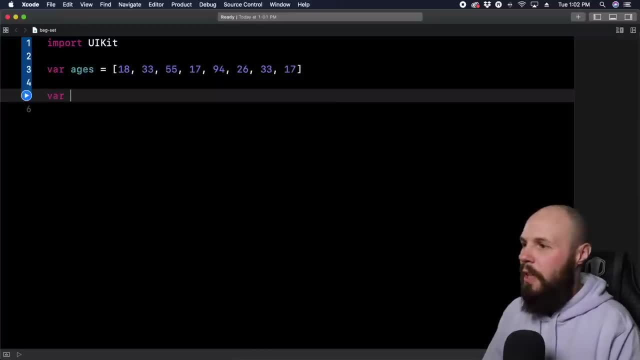 Now to initialize an empty set. this set is a little bit different, So you have to do ages. Let's call this ages set, just to be clear here, And for the array. if you remember, we would do this for the array. 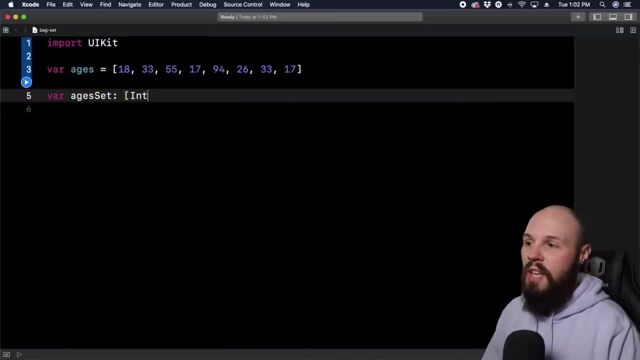 So we would say it is an array of ints when we were declaring a type. Well, for a set you got to be a little bit different. You have to say it's a set and then use angle brackets and you put the type in the angle brackets. 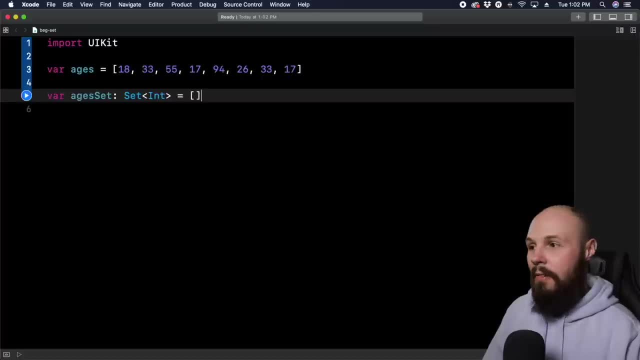 So equals that. So now that is an empty set, right? We've declared here: this is a set of type ints, That's, if you want it to be empty, You can also initialize a set based on an existing array. So that's what we're going to do down here. 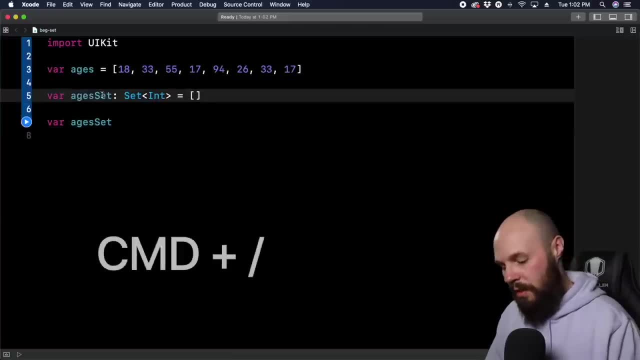 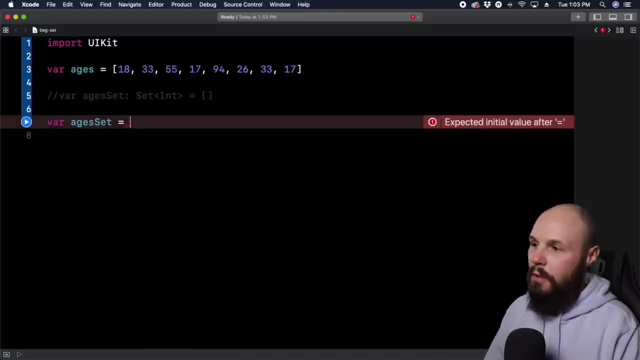 Our ages set. Now I can't have two things of the same name, So let's comment this out. You can do command slash to comment that out. So ages set And now we can initialize this based on an array. So we can do sets and then we can pass in an array. 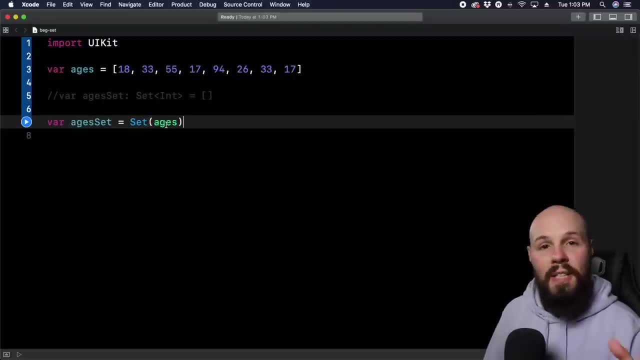 So we can do ages right, So you can create a set based on an array that already exists. This ages array already exists up here. Now, if you remember, I said you can't have duplicates and it's unordered. So what we're going to do is we're going to go ahead. 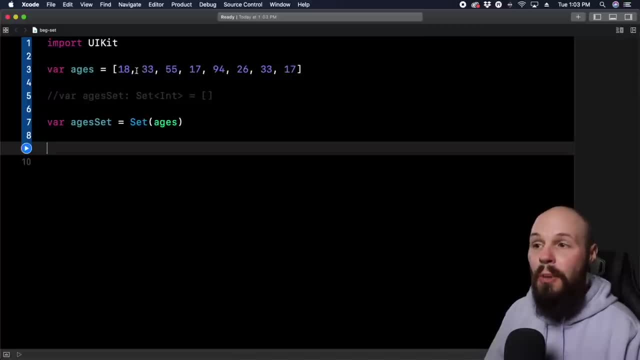 and print ages set And then you're going to see that our duplicates aren't in there, right? If you look here, we have 17,, 17,, 33,, 33, right, We're not going to have those duplicates. 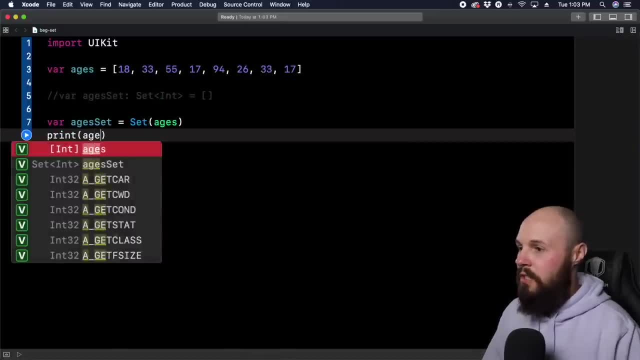 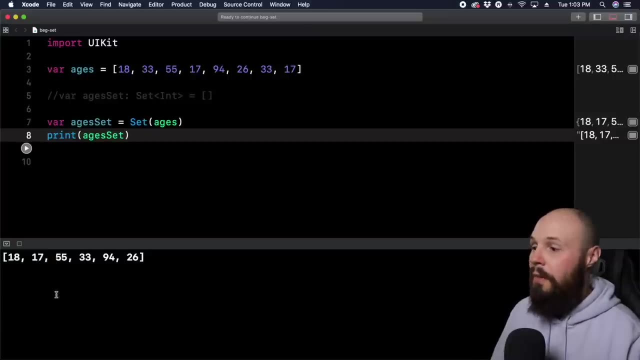 So let's go ahead and print ages set. Print ages set, run it And down here I'm going to move this up. See, we don't have a duplicate of 17.. We don't have a duplicate of 33.. 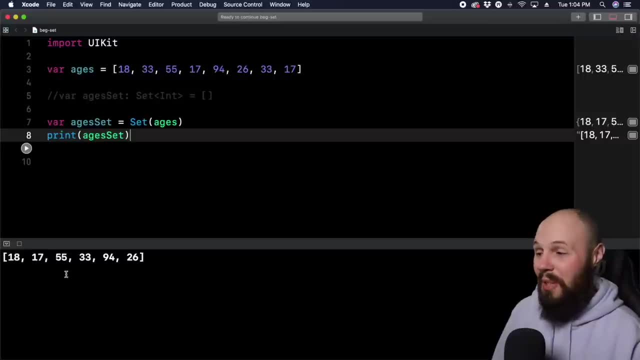 And if you look, it's not really in the order that we have. It's actually kind of close, So I can see where you might confuse that, but it's not in any order. If I run this again, we're going to get a different order. 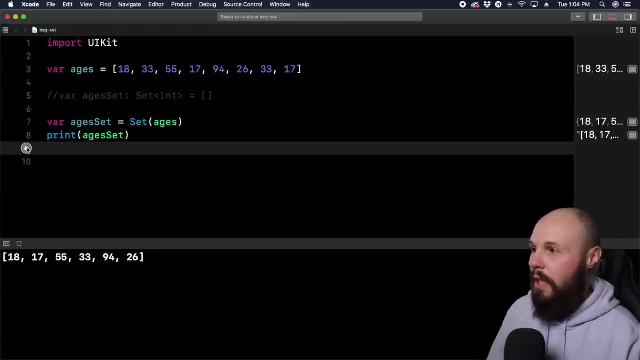 Just pay attention, It's 18,, 17,, 55. So run it again. Well, let's stop it, Run it again. See, now we've got 55,, 26,, 33.. So again, order is not guaranteed. 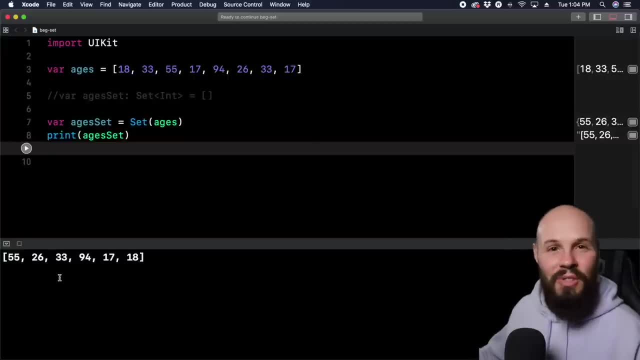 You can't have duplicates. So again back to the question: why would you use a set? Well, it's because of performance. Again, like I said, the set has very fast insertion, very fast lookup, very fast deletion, And the reason being is because, in order for something, 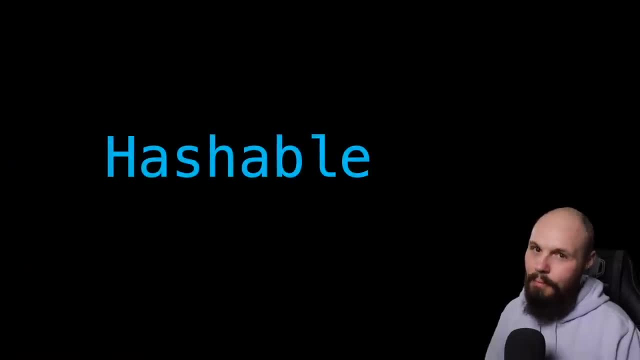 to go into a set, it has to conform to hashable Stick with me. I know as an absolute beginner talking about hashable and hash values and constant time lookup. that is getting a little bit excessive. I understand that. but I can explain it pretty simply. 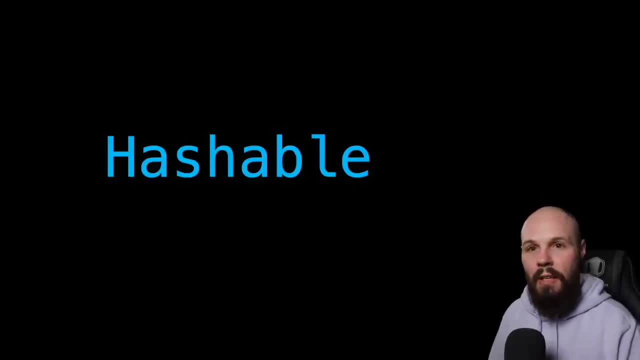 Now conforming to hashable is a requirement to go into a set Now. luckily, the basic types that come with Swift that we talked about, you know, string, int, boolean, double float, those all automatically conform to hashable. 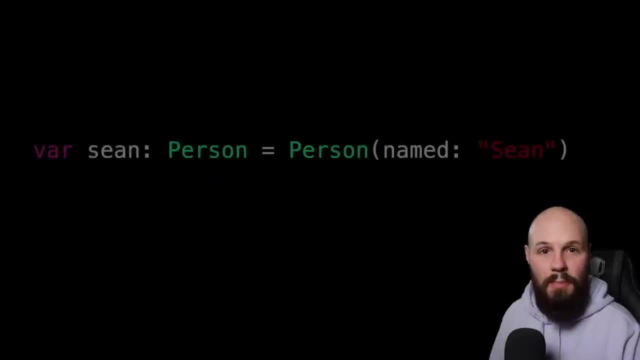 So this is really only going to come into play when you're creating your own types, right, Like we created our person type. Remember that example: you know person with the name Sean that's not going to conform to hashable unless we actually implement that ourselves. 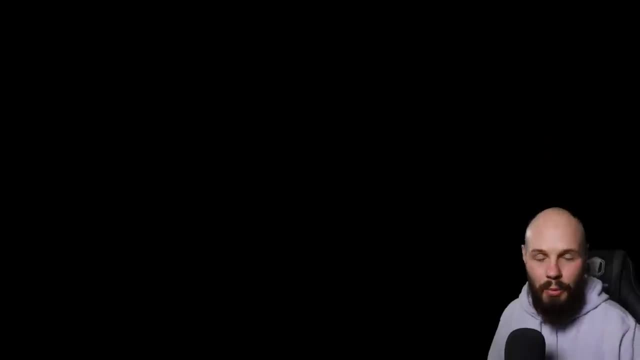 So, until you're building your own custom objects and custom types, pretty much everything is going to conform to hashable, so don't worry about that too much. Again, as long as you're using int double bool string, which is what you'll be using most of the time, 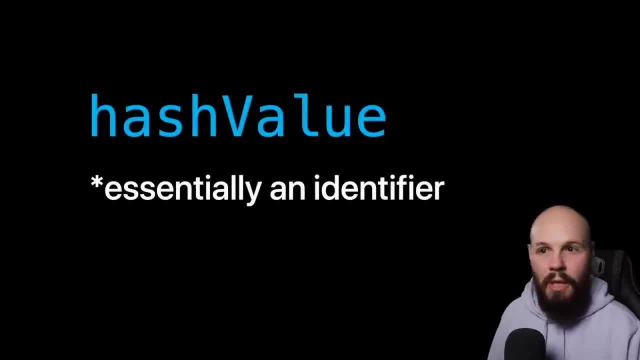 Now by conforming to hashable. what that means is that it just has a hash value, that is, an identifier. Again, I'm putting this super simply: Think of a hash value as, like a direct pointer to that location. Let me do an example to illustrate that. 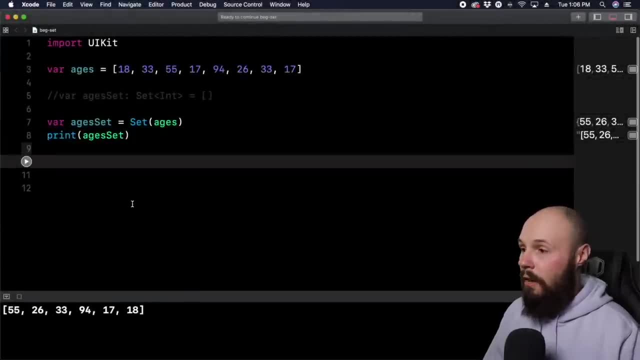 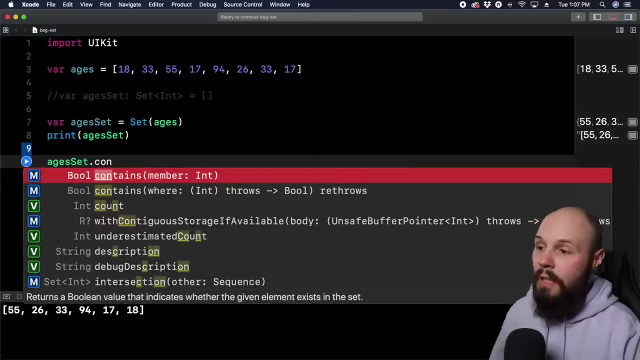 So here back in our code, we can do the contains function here. So we can do ages set dot contains right And you can see the member is an int right, Because this is a set of ints. So I want to see if it contains a certain number. 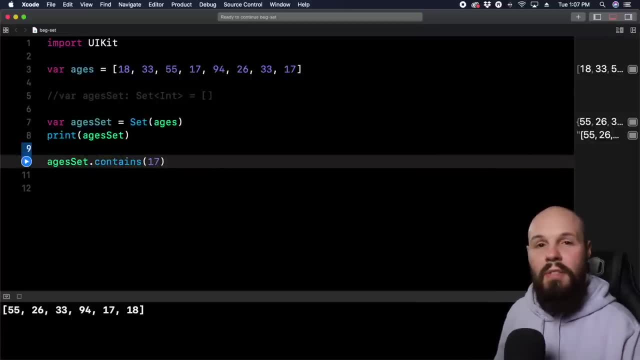 So by doing 17, it can look right for 17.. That's constant time lookup, Whereas, you know, array also has a contains function. However, what an array has to do- and this is why a set is faster- an array would have to go. 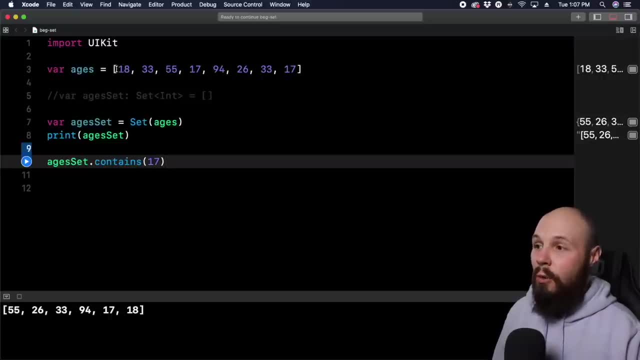 it would have to check the whole array. So if I was looking for 17 in the array of ages up here on line three, what the array does is it's going to check here It'd be like 18.. Nope, that's not 17.. 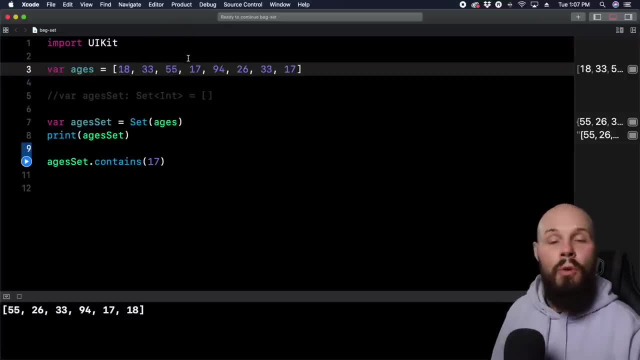 It'll check 33.. Nope, Okay, It'll check 55.. It'll check 17.. Okay, cool, Now in an array of eight items. no big deal, But you can imagine. you know if you're storing data. 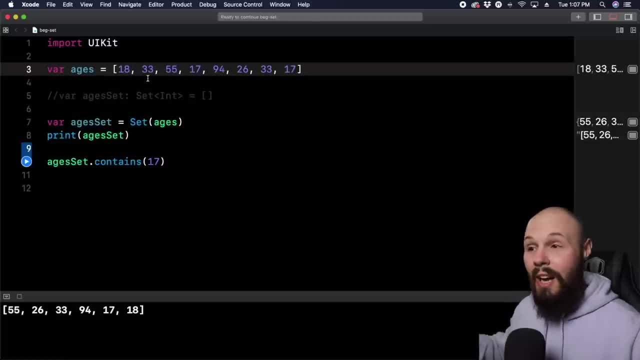 you can have an array of, you know, a thousand, 2000,, a lot of numbers, items. So that's where the performance comes in, where, again, the array has to look through the entire array until it finds the number Whereas a set, because of the hash value. 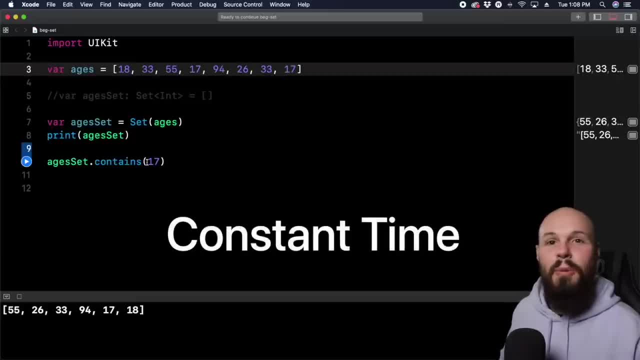 can go right to that numbers And that's called constant time lookup. but basically what that means is the time to look it up will stay the same no matter how big the collection gets right. So if our set it has a million items in it. 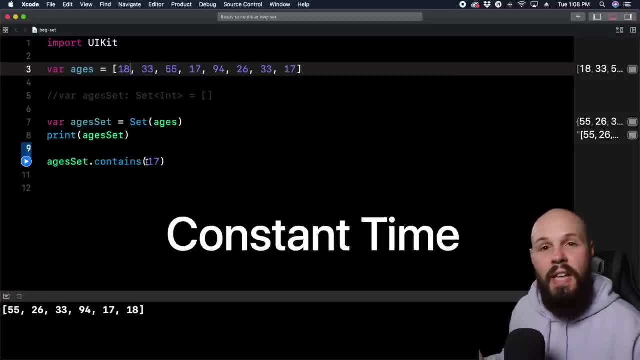 the time to find 17 is going to be the same exact time as if our set had 10 items in it, Whereas the array is different. right, If the array has 10 items, okay, that's going to happen pretty quick. 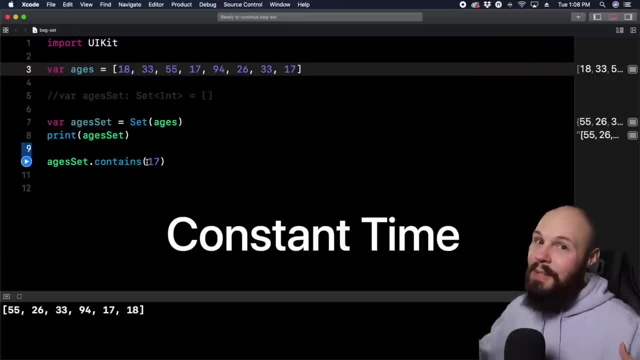 It only has to check 10 items. If the array has a million items now, it's not going to be as quick because it has to check through a million items. So hopefully you're starting to see the performance of a set. but again, it's a trade-off, right. 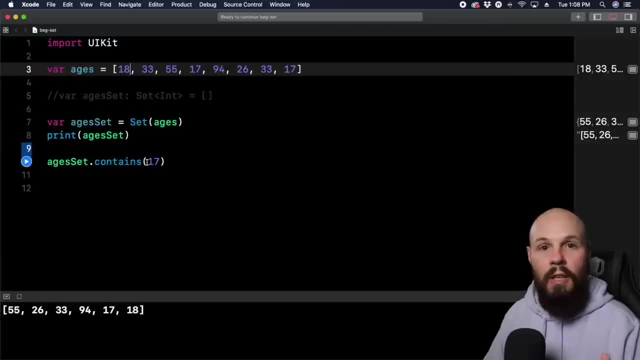 A set gets that performance because they don't guarantee an order and they can't have duplicates. So that's the trade-off: They trade those features for performance, Whereas an array- you can't have duplicates- It's always going to be in the same order. 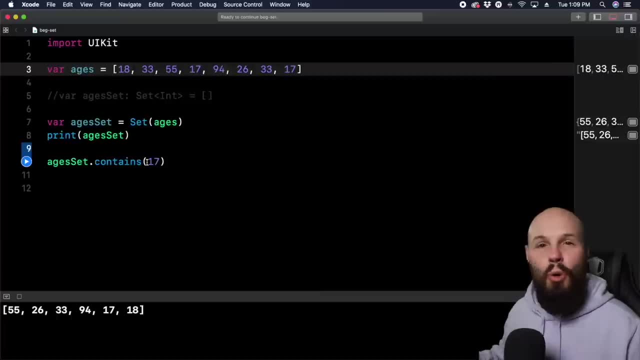 but it's a little less performant And that's actually a good analogy for programming in general. You'll find as you go throughout your career, when you're making decisions on what to use, it's all about managing the trade-offs, right. 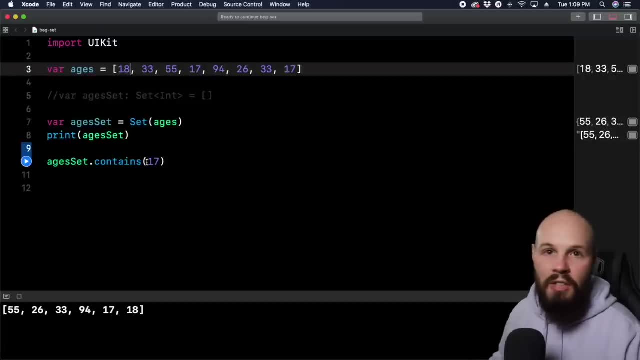 Every approach and implementation has pros and cons and it's all about choosing the right tool for the right job based on those pros and cons. So let's run this and you should see it'll print true Here over on the right. yep true. 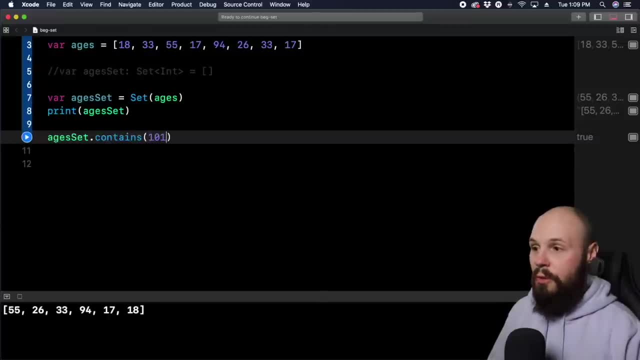 because it does contain 17.. Now if I want to say, does it contain 100, which we know it doesn't, or 101,, my finger slipped. it'll come back and print false because it does not have 100 in there. 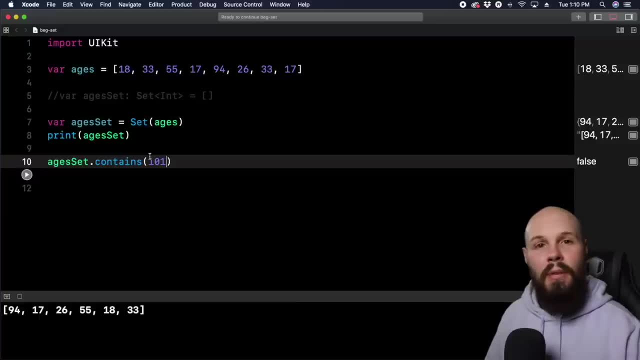 So that's how you can see if your set contains a value. Now let's talk about inserting a value into our set. If you remember, on our array we used append and that tacked it onto the end of it because it keeps the order the same. 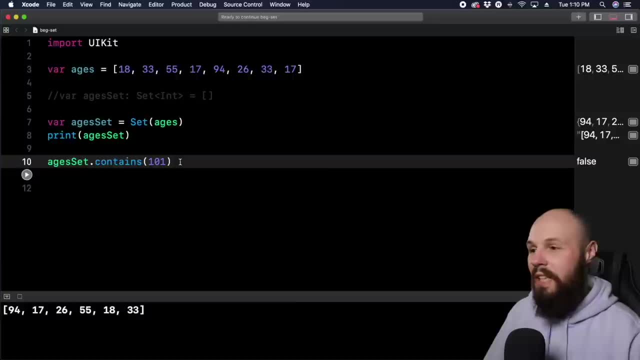 However, sets don't have an append right. We just insert it into the set. It's kind of like throwing it into a bucket, Like we don't care about the order, Mix it up, who cares? We're just throwing it into that bucket. 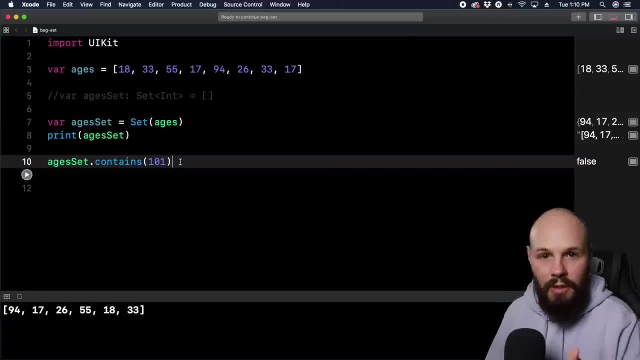 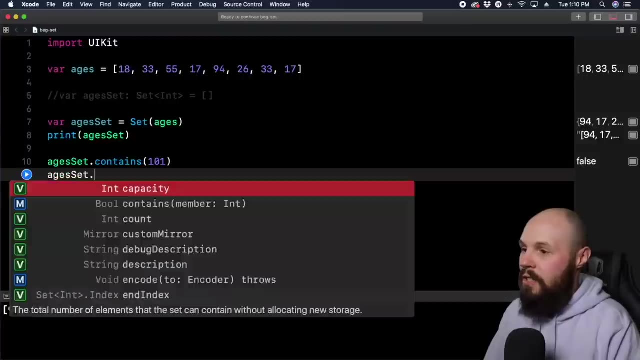 And again, that's the whole. you know very fast: insertion or deletion. I don't have to pick where exactly I want to put it. We're just putting it in the bucket with everything else, And to do that you can do ages setinsert new member. 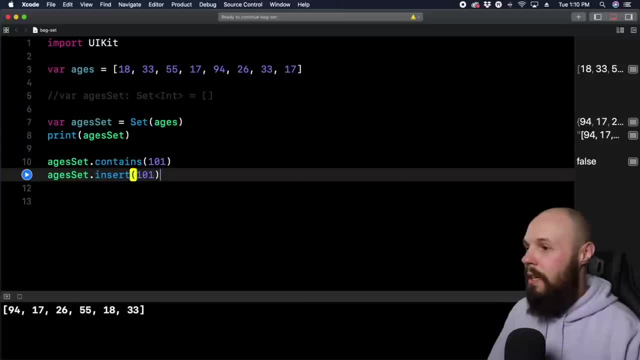 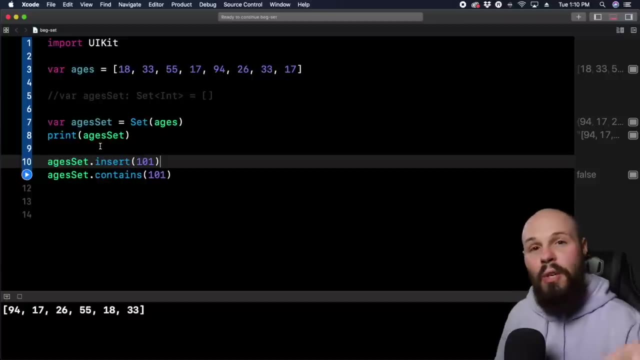 And you can see we want to. let's insert that 101 that we put up there. And because the code you know runs down the line here, let's cut this and put this up here, So that way we're inserting 101 into our set. 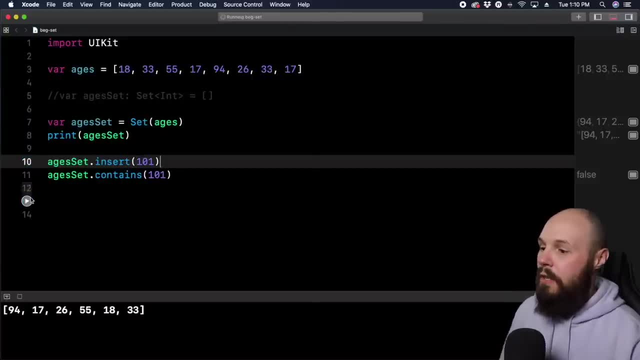 And then we're going to check to see if it contains it. And now you can see down in the printout we have. I got confused because we didn't have a 101 down here in the printout. That's because I printed it before we added it. 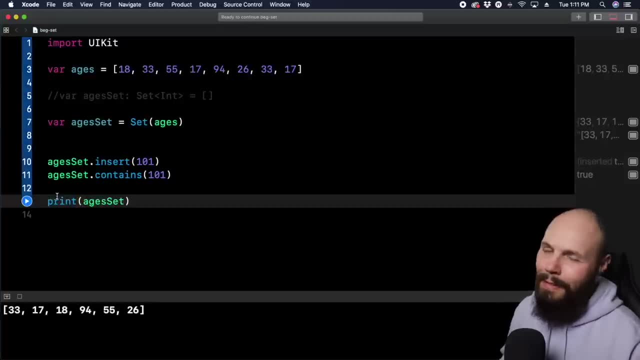 Again, the order you put things in matters, So hopefully that's another little bonus lesson that I didn't intend on. But now we're going to print ages set down here. Now, 101 should pop up in the set. There it is. 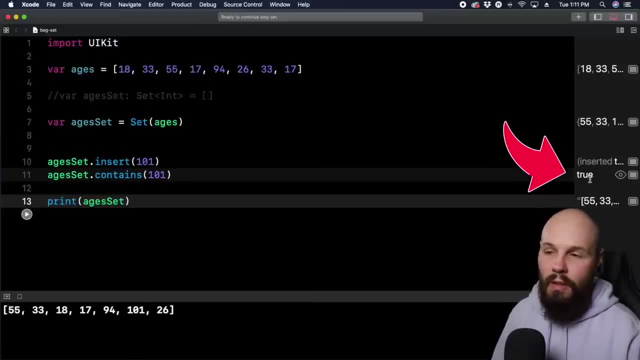 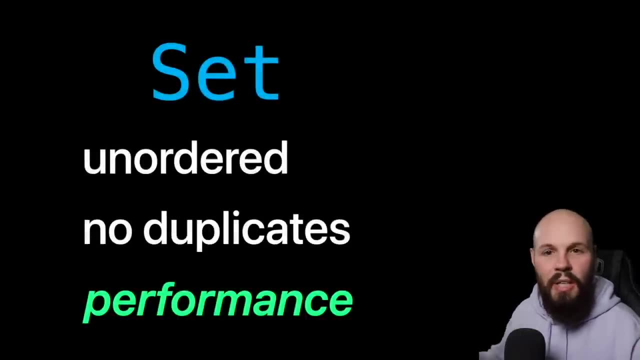 So it got inserted. And then let's check our contains 101.. That is true. So again, to reiterate the main differences between sets and arrays, even though they're very similar because they're a collection of items, is that: 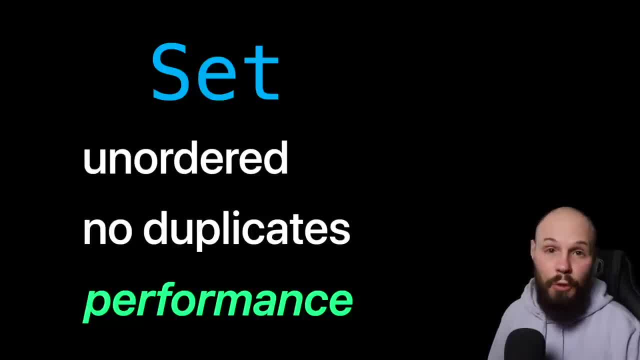 sets are unordered, arrays are ordered. arrays can have duplicates, sets can have duplicates and sets have faster, you know- insertion, removal lookups because of the hash value requirement And again it gets that performance boost because of the trade-off of no duplicate values. 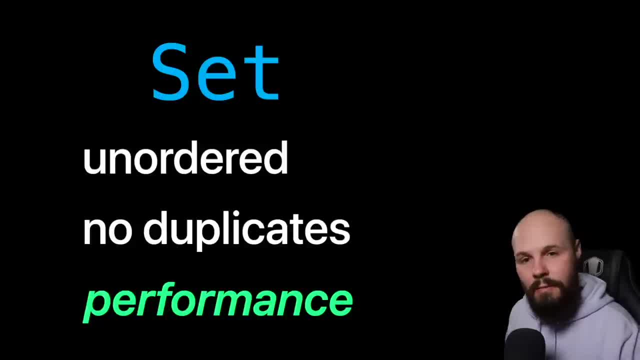 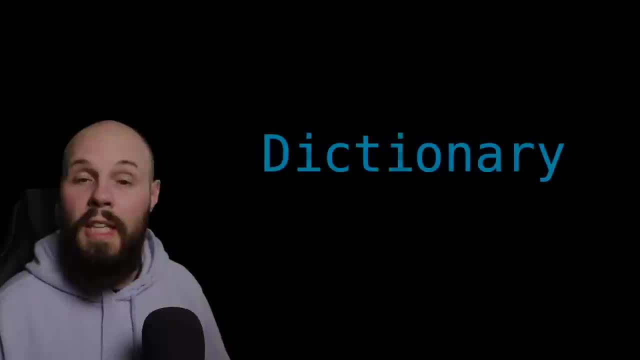 and not having to worry about order. So that wraps up the basics of a set On to the next collection type and that is dictionaries. Our third collection type that we're going to discuss is a dictionary And just like a set in an array, 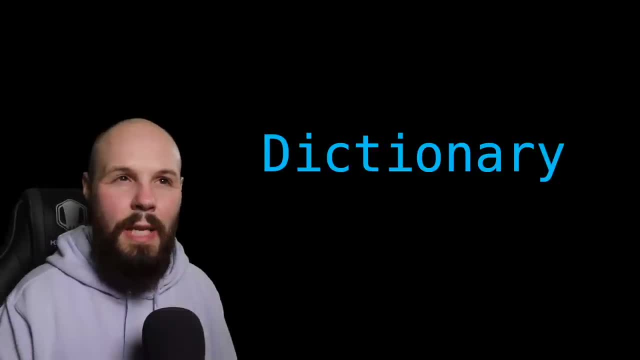 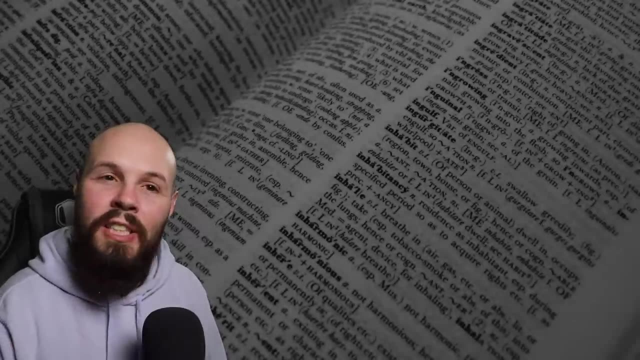 it is a collection of items. except this collection of items has labels, kind of right, They're called key-value pairs And if you think about a dictionary, like what the title is right, In a dictionary you have the word: 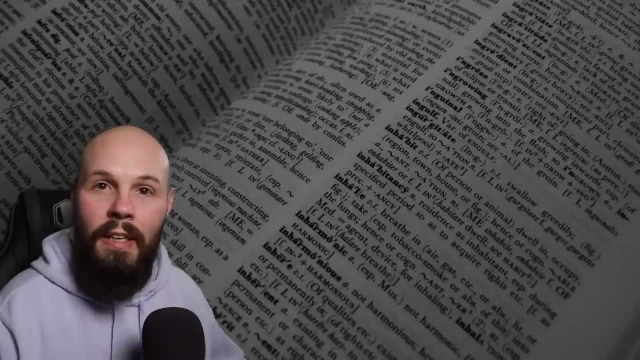 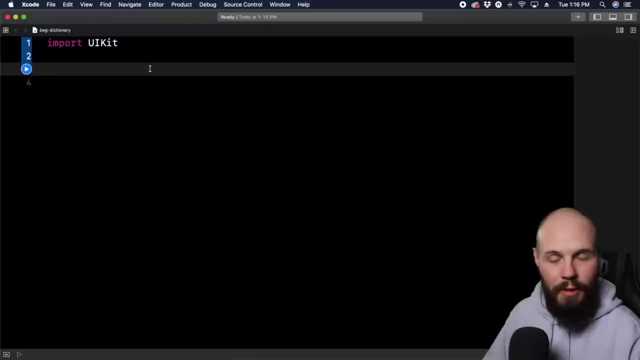 and then you have the definition right. So think of the word as being the key and the definition as being the value in the key-value pair. Let's dive into some code for an example. Now again, here we are- blank playground. 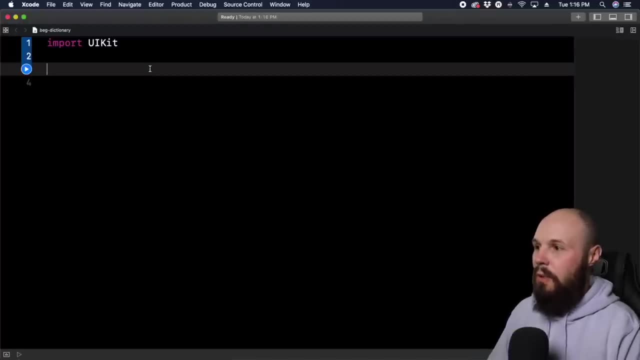 Go ahead and create that for yourself, But we're going to create a dictionary called devices. So let devices and our dictionary is going to be of type and you'll see how we declare it here. It's going to be a type string. 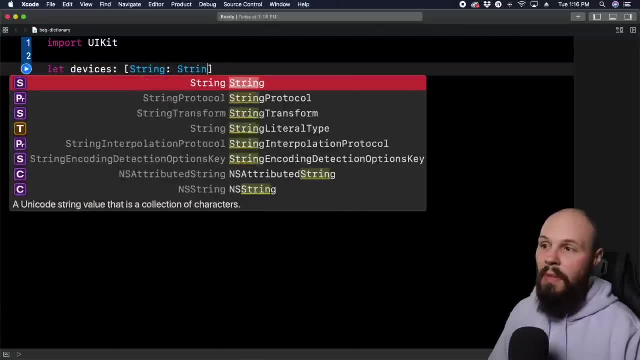 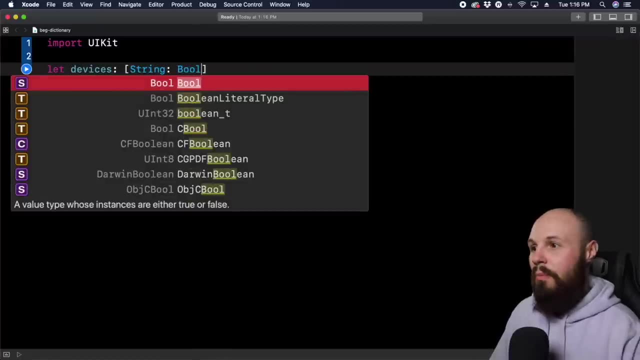 because a string is going to be the key and the value is also going to be a string. This could be an int or it could be whatever you want, a bool, depending on what type of dictionary, But because I'm having the names of my devices. 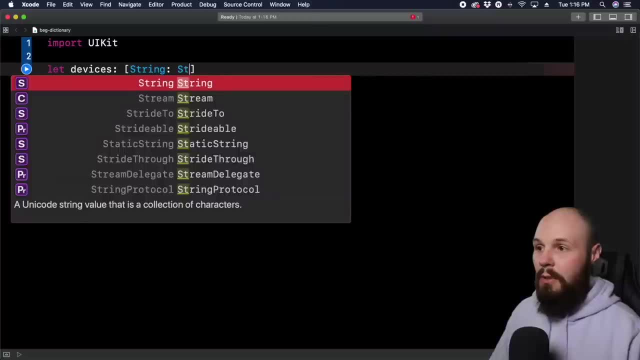 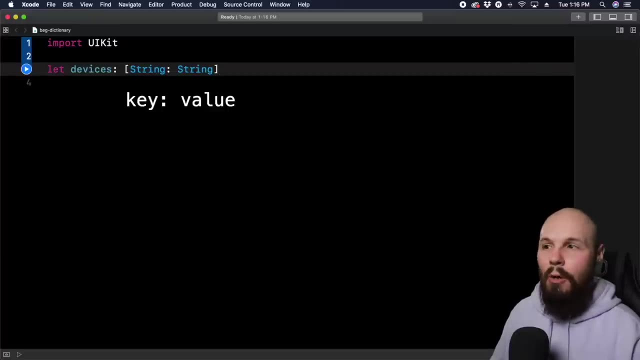 like my computer, my phone. this is also going to be a string, So you have to declare what type your value is. Your key is almost always going to be a string. It's kind of the standard. Now, you know, there's some situations where maybe not. 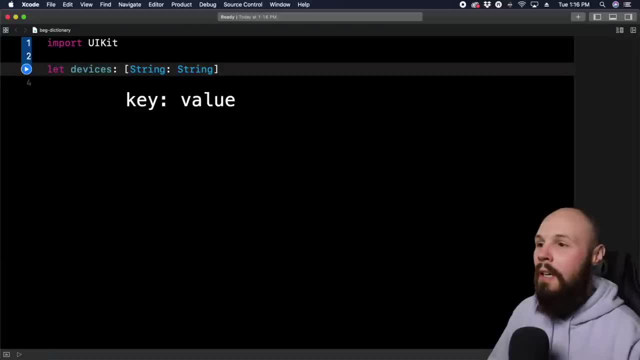 but, but 99% of the time your key and the key-value pair is going to be a string, So that is going to equal. right now there's going to be an empty dictionary, So you do the square brackets and then the colon in the middle. 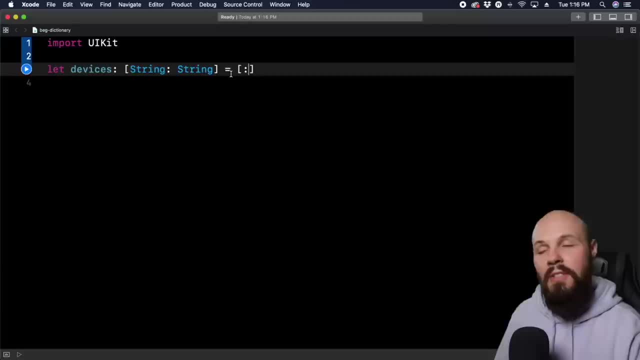 because, again, the colon separates the key and the value. right, The key is on the left of the colon, the value is on the right of the colon. So let's put some values in here And, as you can imagine, if I listed out five values, 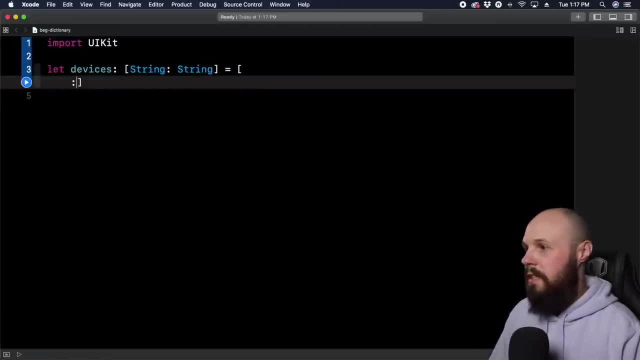 this is starting to look weird, So we're going to go and put this on next lines here. So for the first key, let's do what is my phone And the value of the phone is going to be iPhone, is going to be iPhone X. 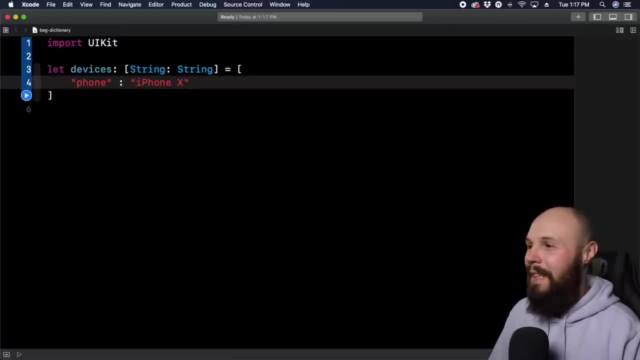 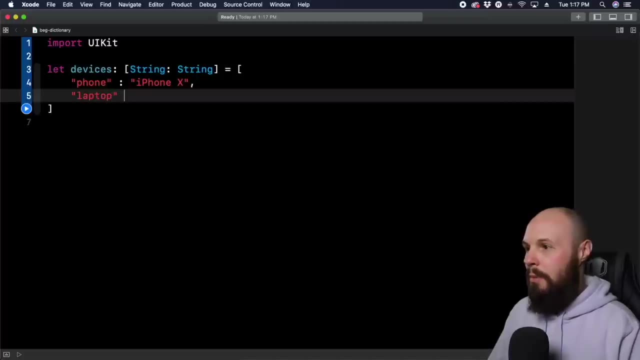 Yes, I call it an X and I still have the X. I'm waiting, waiting to upgrade, And then these are comma separated. So now the next key is, I don't know, let's say my laptop, the laptop, and then you shouldn't have a space after the. 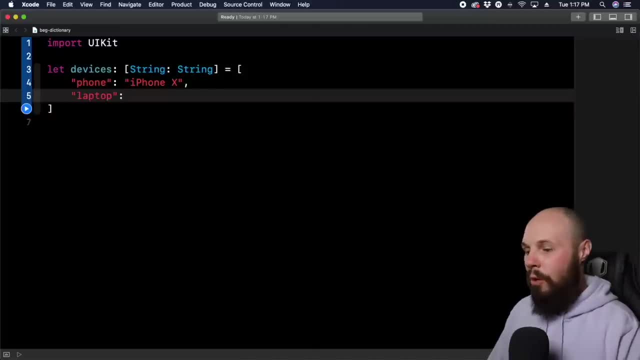 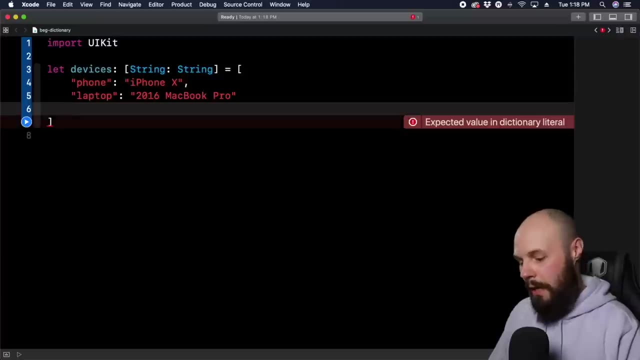 after the key, It's a little style preference. So, laptop colon and that is a 2016 Mac book pro, And then we can do, you know my, what is my, what is my tablet. I'm only going to do four of these a tablet: 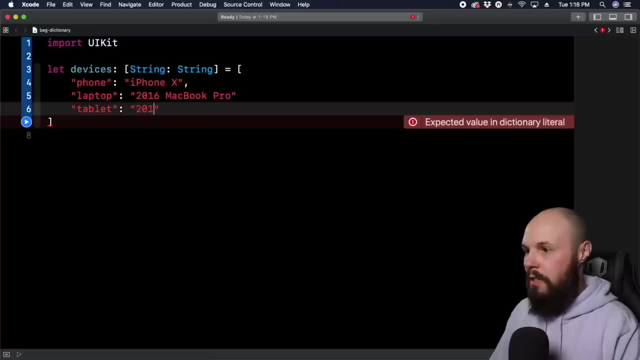 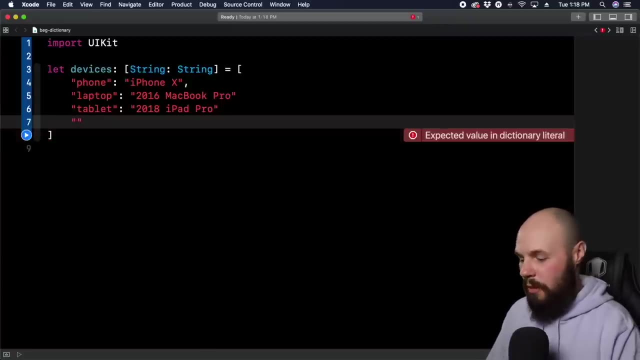 And colon. so that's the key and the values- is the 2018 iPad pro, And then we'll do desktop right. So these are- I'll kind of put this into context here once I'm done typing this. So, desktop and colon is a 2017 iMac pro. 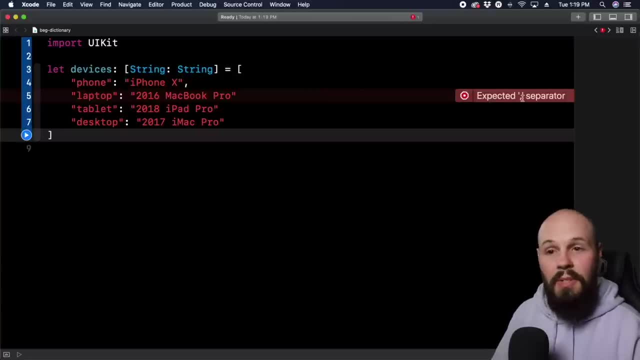 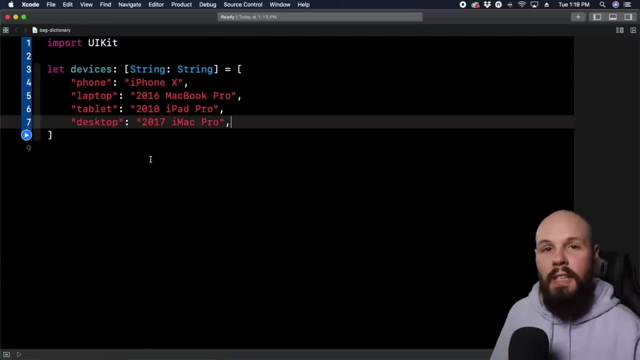 Okay, So these are my devices. Whoopsie expected a comma separator. I'm getting that error. I always forget to do this. These need to be comma separated. So this is my dictionary And, like I said, it's a key value pair. 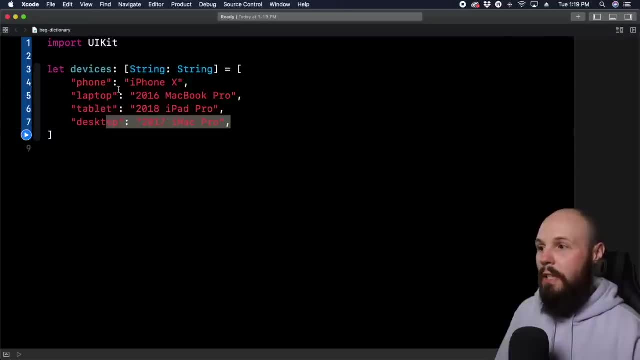 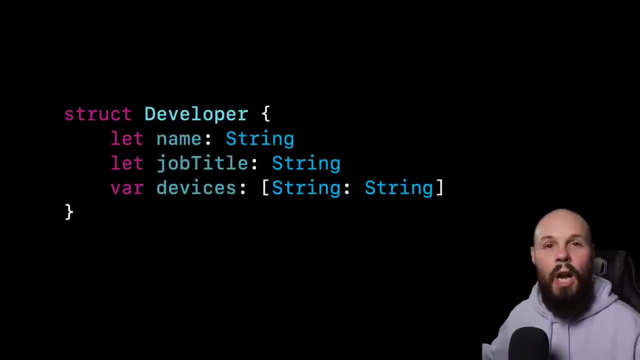 So you can see the key- phone- laptop, tablet, desktop- and then the value is whatever the value is. Now to put this into context, let's say we had a developer object. We're going to get into classes and objects later. 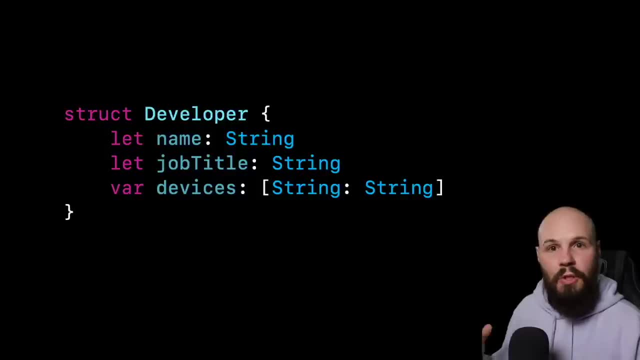 but you can imagine like an object, say the object is developer. Well, your developer has a name. Maybe your developer has a job title, and then your developer may have a dictionary of devices attached to it, So you know what devices your developer has. 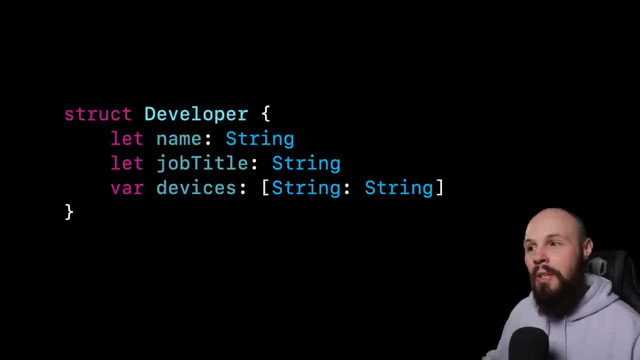 Again, that'll all make sense when we get into the classes and objects part of the course. but that's a little preview. You can kind of get your mind going And that direction. now to access values in our dictionary, we need to look it up through the key. 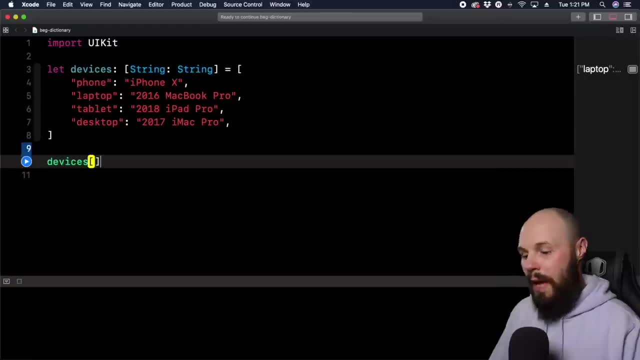 So let's do devices and in the square brackets you just pass in the key of what you want. So let's say we want our laptop. So if I run this, we'll see on the right over here, see 2016 MacBook pro, because I accessed the laptop. 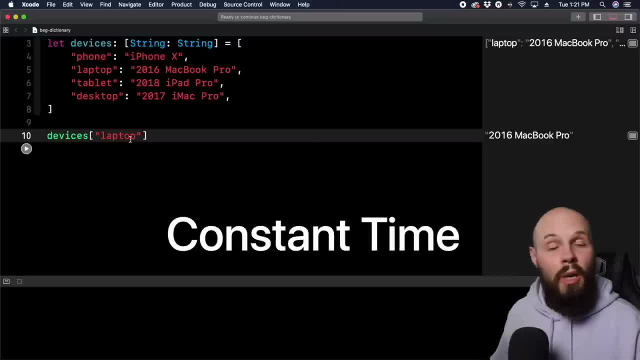 So by passing in the key I can get the value. This is also constant time lookup, So this is a benefit of dictionaries. They're very fast because you have the constant time lookup similar to the set, And the way that works is we know the key. 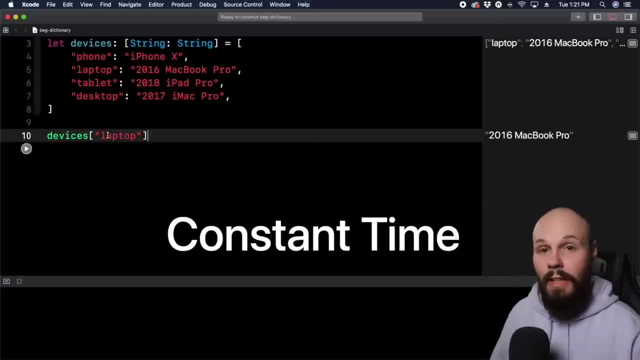 so we go directly to that key and get the value right. Like an array, We don't have to look through all the values to find what we're looking for. Like we know the exact location of what we're looking for And that location is based on this key. 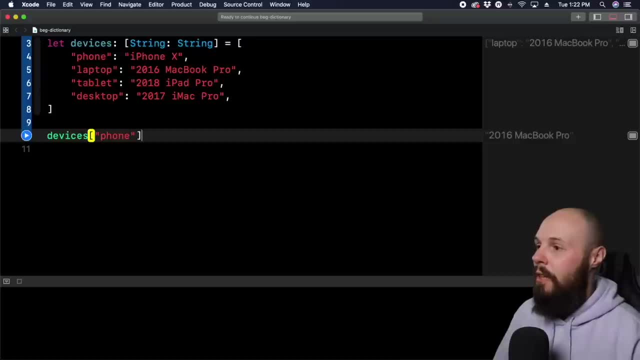 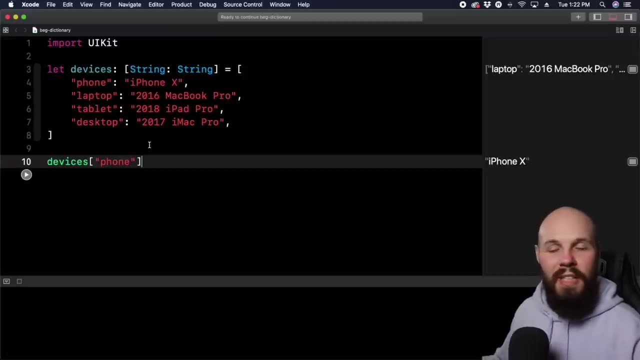 right. So just to prove this here, let's do phone. What kind of phone do I have run it over here on the right iPhone X, not iPhone 10, iPhone X. So that is a basic example of using dictionaries. Again, it's a good way to store a collection of information with, essentially, labels on. 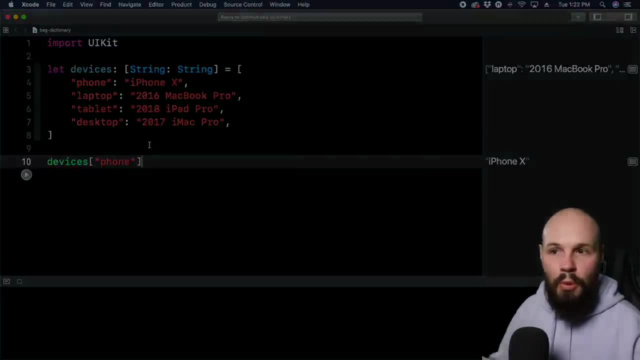 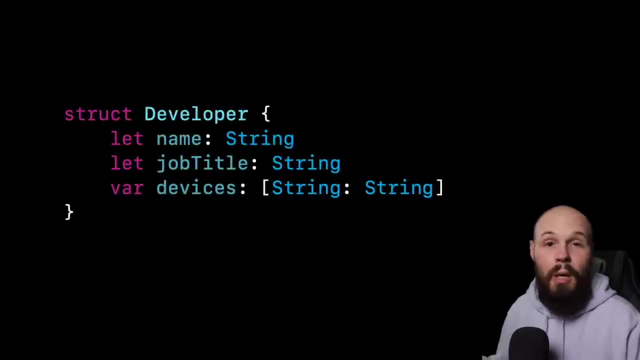 it Using the key value pair. again back to our real world example. if we have our developer object right, A developer would have a name. That name would be a string. developer would have a job title. That job title is probably a string. 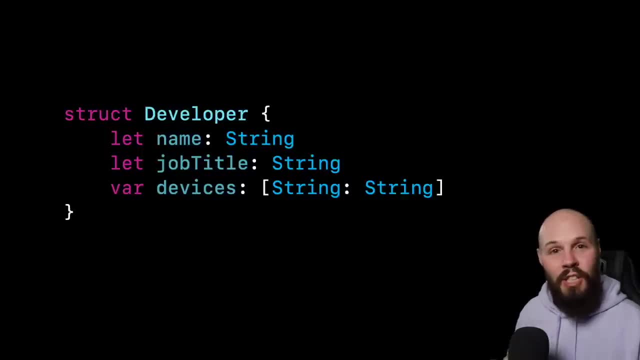 A developer would also have devices. but except, devices is going to be a dictionary. So we can see: Oh, the phone is the iPhone, The laptop is the Mac book pro, et cetera. So that's the basics of dictionaries. onto the next video. 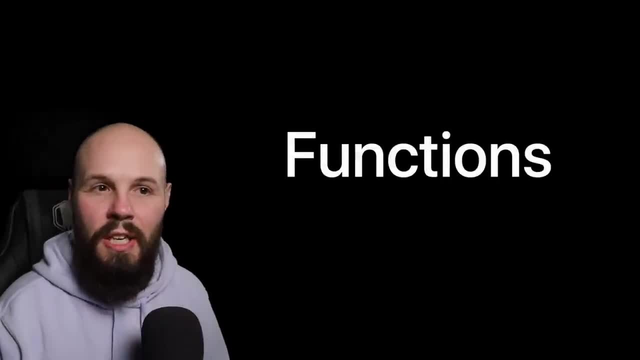 All right Onto one of the most important topics, And that is functions. Think of functions as like a compartmentalized set of instructions right That you can reuse throughout your code base, And they can range from very simple one line functions to pretty complex. 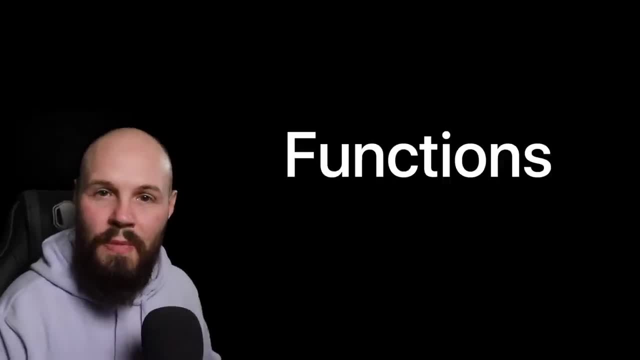 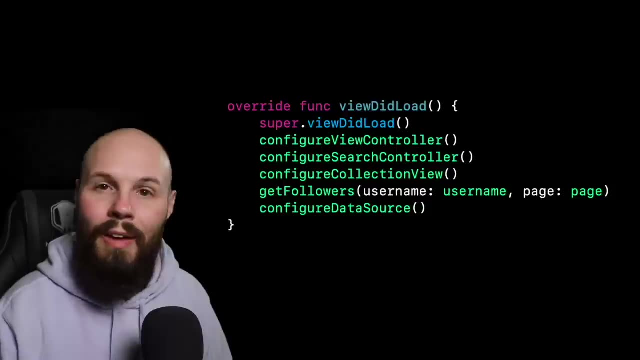 multi-line functions. Let me show you a real world example and then we'll dive into some basic code examples. So here on the screen you see an example from my take home project app in a view did load. We haven't gotten to that yet. 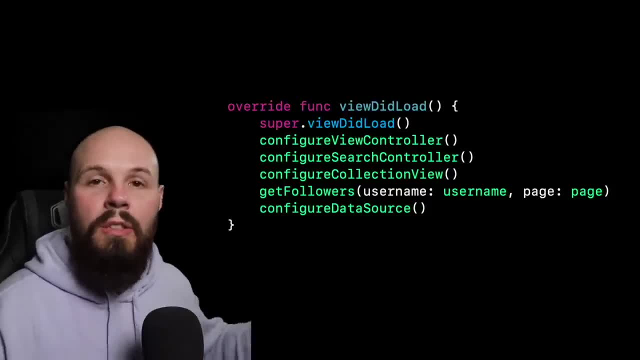 but view did load gets called when a screen of your app gets loaded. So essentially, what's going on here is this is a list of commands as to what's going on on this screen. As you can see here, it's configure view controller. 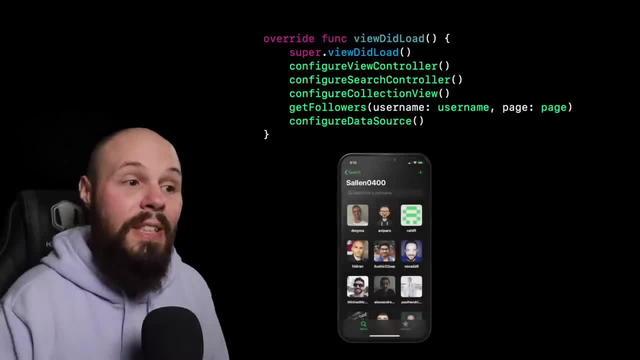 configure search controller, configure collection view, you know, get the list of followers based on this username And then we're going to configure the data source. So you can see, those are all functions that are being called, but that's just what we're actually using: the functions. 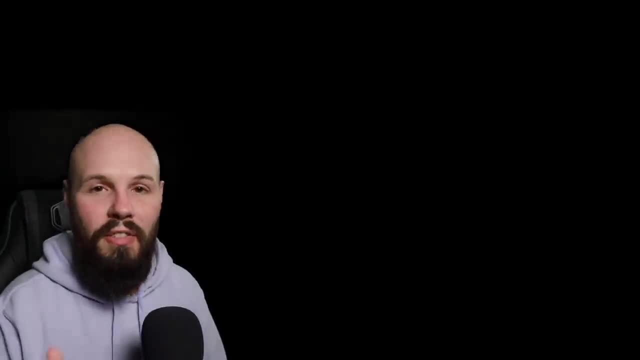 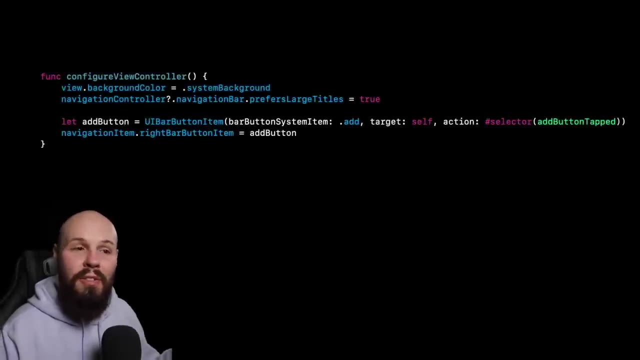 That's not where we defined the function. Let me show you one of these functions definitions. Here's where we actually wrote the function configure view controller And you can see in this function again, it's a compartmentalized set of instructions. 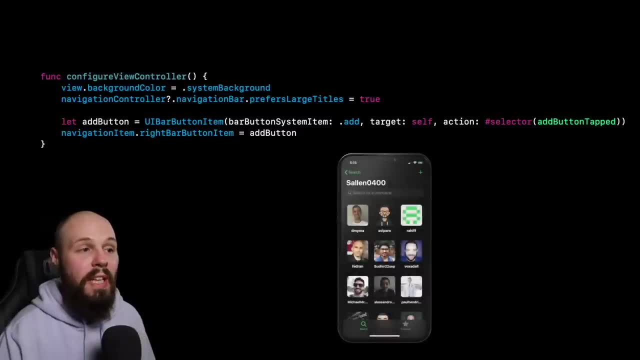 right. So how we're configuring our view controller is: you can see we're setting the background color to system background. That's just white or black based on dark mode. We're configuring our navigation controller to show large titles. I understand a lot of this is probably a different language to you. 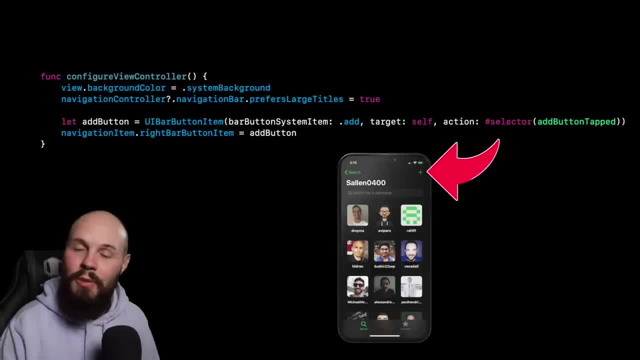 but I'm just showing you an example. We're creating an ad button. If you ever use an app that has like a little plus button at the top, that's what we're adding here. And then we're putting that ad button into our bar button. 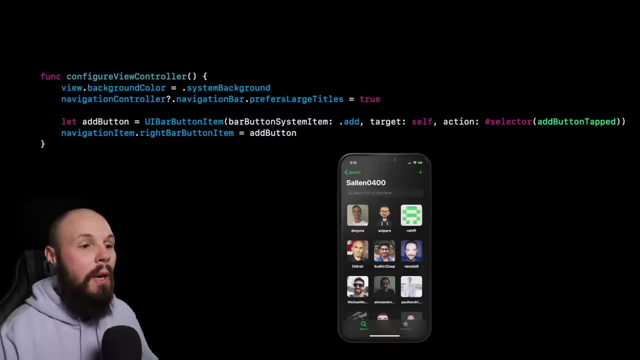 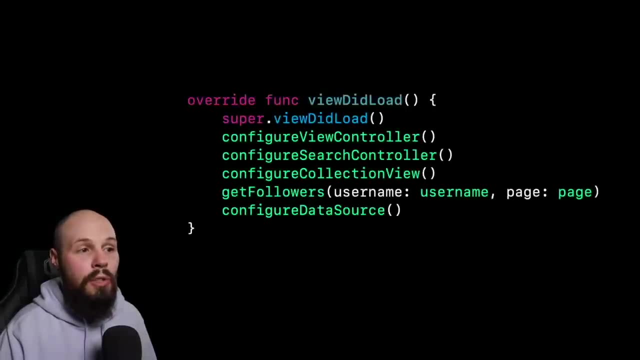 I'll show you a picture of the screen here to show you what's actually going on. But the point is, you can see, you can have all your logic inside this function where it's defined, And then now you can use configure view controller wherever you want in your code here. 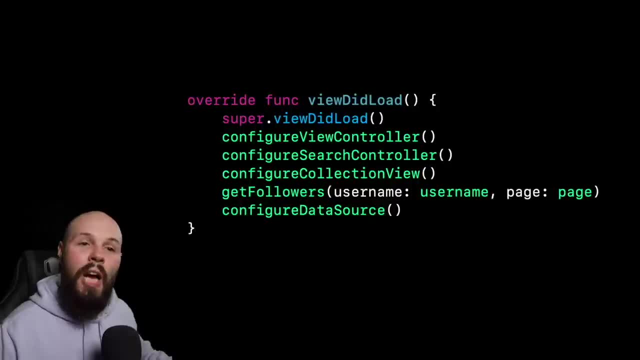 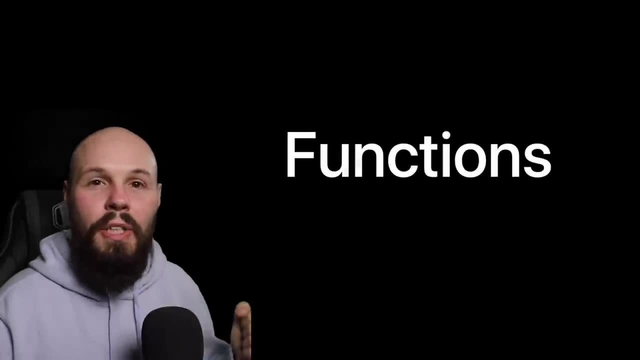 We happen to use it, you know, in view to load when our screen first views. that's how we're configuring the view controller And you can see we're calling it in view to load. So again, to reinforce that it is a compartmentalized, reusable chunk of code. 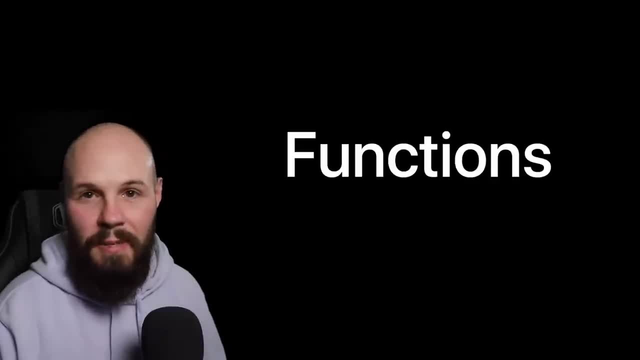 right. So you can see how we define it and then how we use it once it's defined, All right. So that was a real example from an actual app, So don't worry if a lot of that went over your head. we're going to dive into some basic examples that will hopefully connect the 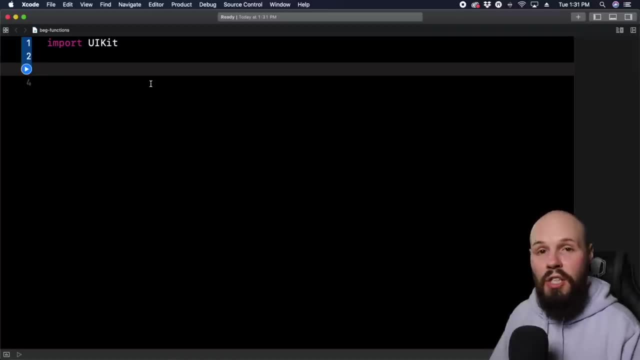 dots for you, All right. So let's start off super simple. In order to to clear a function, you have to put the keyword funk in front of it, short for function. So F, U, N, C and let's say a print instructor's name. 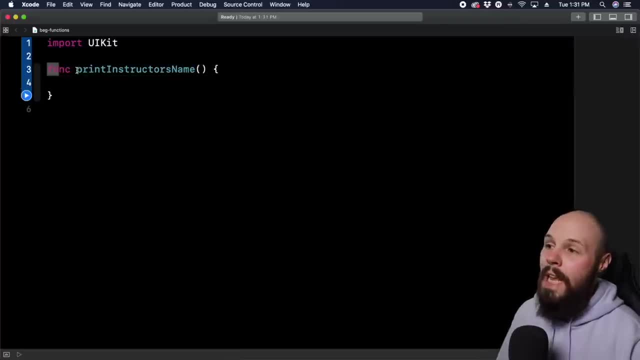 right. So what you do here, you have the funk. here You have the name of the function again print: instructor: instructor's name. Now, the name of the function should always be a verb, right, It shouldn't be a noun, Like you wouldn't want to do, just a instructor's name. 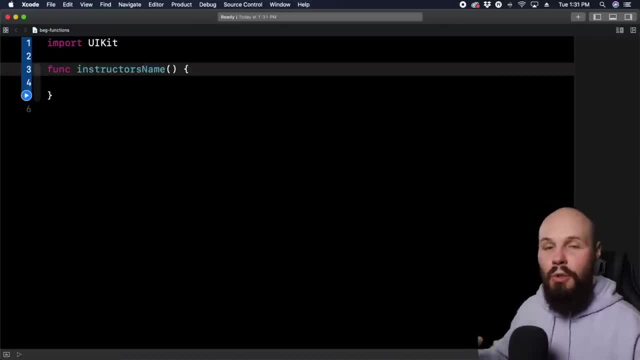 right, That's a noun, Because a function does something You want to. you want it to be a verb, So it should always sound like it's doing something. So print instructor's name. That's a verb, It's doing something. 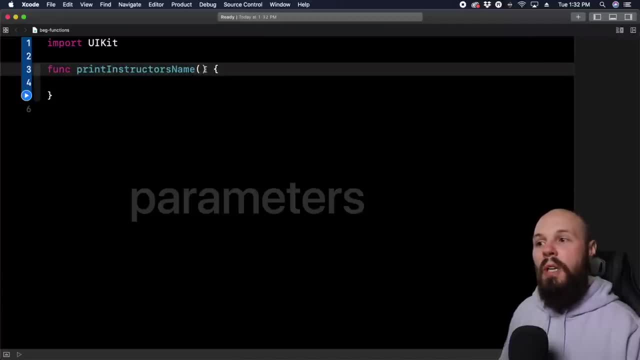 And then all functions need to have these open and close parentheses at the end. This is where a potential parameters come into play. more on that in a future example. For now we don't have any parameters and then you do an open curly brace in a. 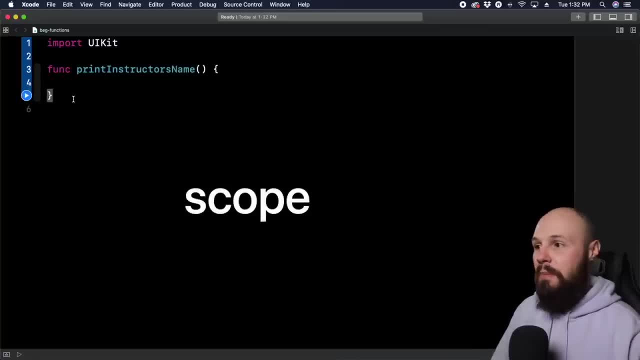 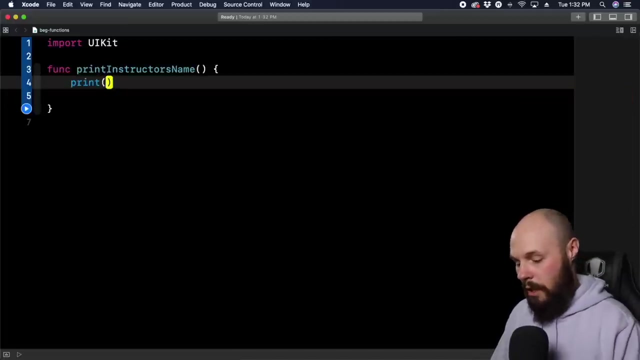 closed curly brace. This defines the scope of a function. So the scope of the function is basically everything that's inside this function. And what's inside this function is what's going to be between these two curly braces. in this super basic example, We're just going to do print and put a string in there. 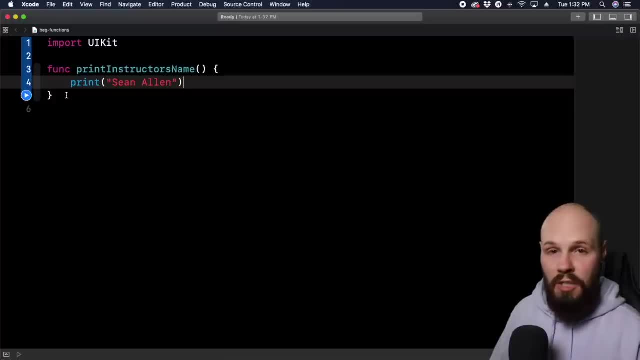 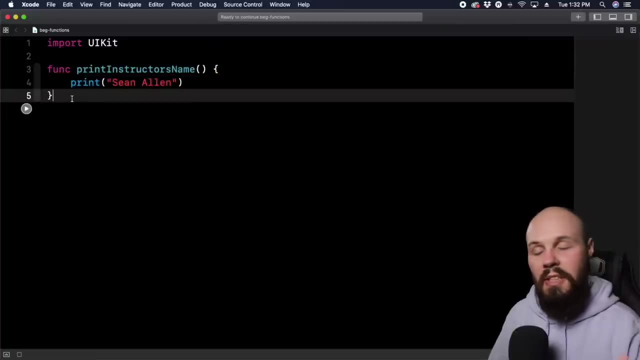 Sean Allen, right now, just defining this function doesn't automatically run it, right? I'm going to run my playground. Nothing happens. You have to call your functions. Remember, just like the example I showed you, we define the function and then we used it. 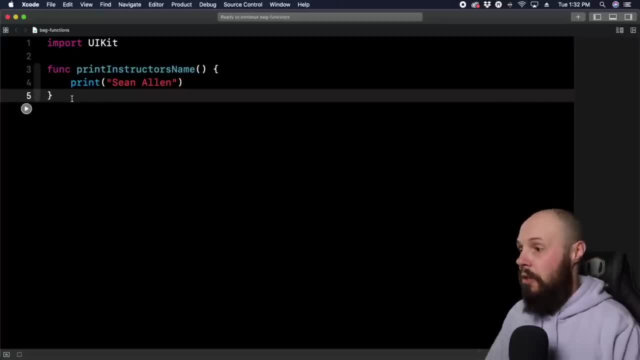 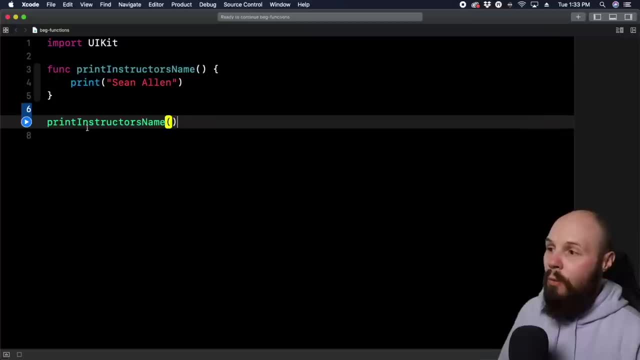 Name right, So you can see there's my function. So now when I run it, this is actually going to get called. So that means print will actually execute. right, You have to call your function in order for all the code you put in there to 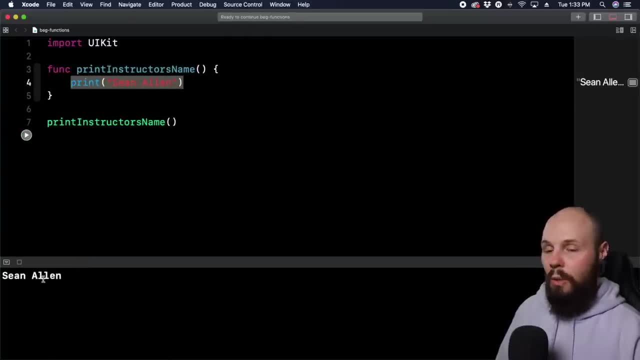 execute. So run it Now. you see Sean Allen in the lower left. So that's the super basic example. There's no parameters, There's no return types. We're going to build on this to show you that. So let's delete this for now. 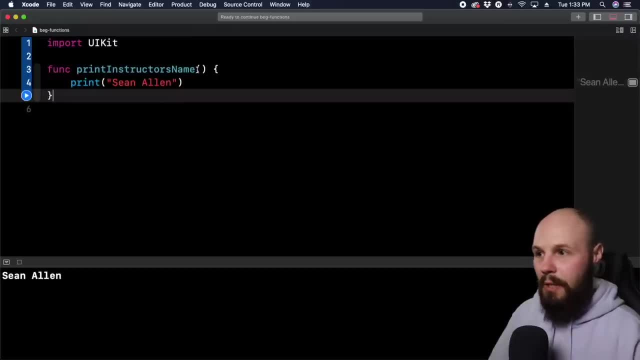 And let's modify our function So it takes in a parameter. Now, like I said, a parameter goes inside these parentheses. So right, We hard coded Sean Allen. So anytime we called print instructors name, it's always going to be Sean Allen. 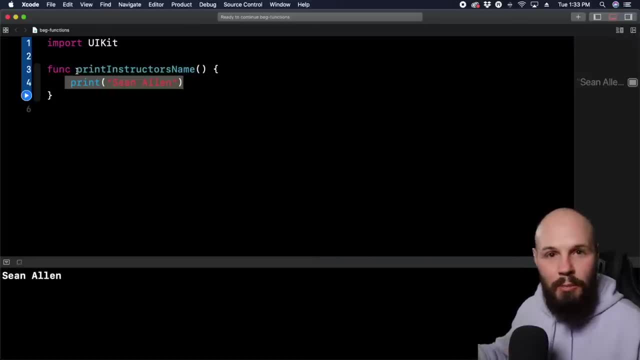 What if we wanted to pass in a name? that way our function could be flexible and reusable. We have to tell it what name to print out. So here we can do: let's get rid of name here in the function. And now we need to label our parameter. 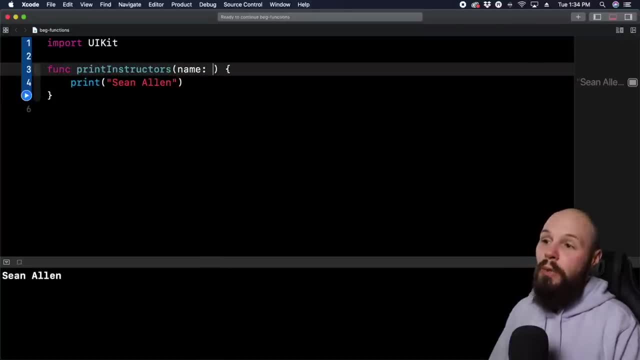 So let's call it name And it's going to take in a string. So let me explain what's going on here. So again, we have the keyword funk to define our function, We have the name of it- print instructors- and then name is the label of our parameter. 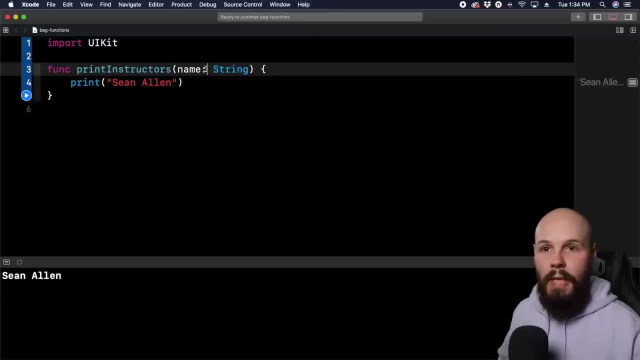 And the parameter it takes in is going to be a string. You have to give it a type right. A name is not an int, It's not a Boolean, It's a string right. So that's the type we're going to pass in. 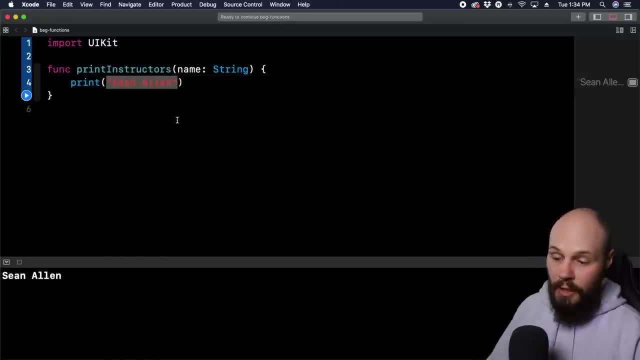 So now, instead of printing Sean Allen and telling it what the print, we're just going to say: print name, right, Cause name was our, the label of the parameter, So we're going to print whatever name we put in, And the name we put in is going to be down here when. 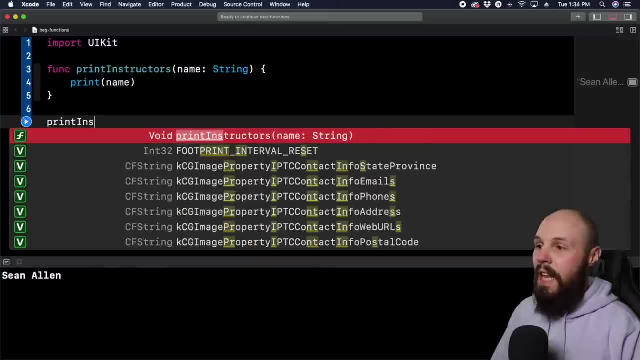 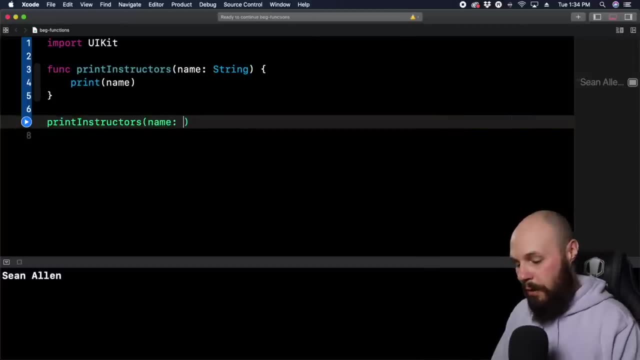 we call it. So now let's do print Instructors name. Now it's saying: okay, in order to call this function, you have to tell me what name to use. So now, and like, like I said, I can't put in five. 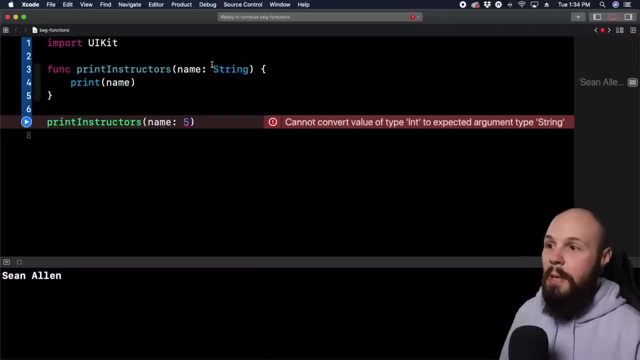 right, It's going to tell me: Hey, no, we expect a string because again we declared the type up here as a string. Again, this is Swiss type safety in action. So now we have to pass in a string. So now let's do, Joe. 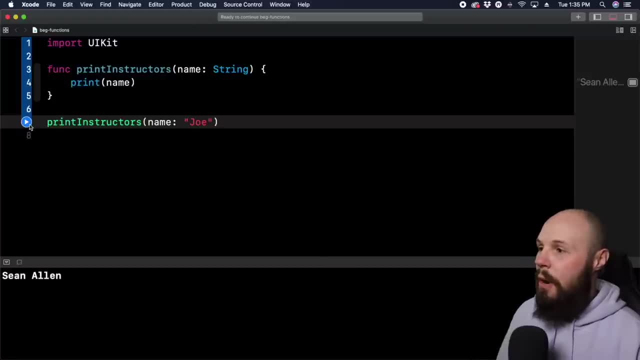 right Now it's not Sean anymore. just to show you that it's not going to print Sean. So now when I run it down here, you're gonna see it printed Joe. So now we're a function up here. It's not always programmed to say Sean Allen. 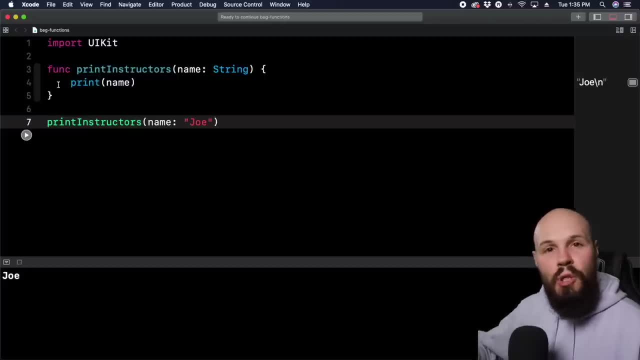 Now we can say whatever name we tell it to be And that's, in general, how you want your functions to be. You want your functions to be super generic so they can be reused in any situation. right, You can imagine we could have print instructors name for Sean. 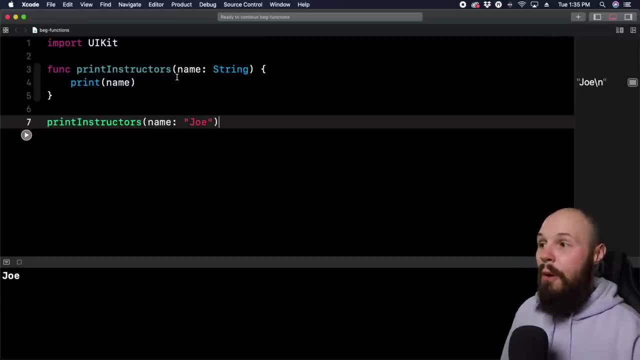 for Joe. you know we could have five functions printing out specific names, but now we just have one function where we tell it what name to print out. And again, name is the parameter and you have to give it a type of a string. 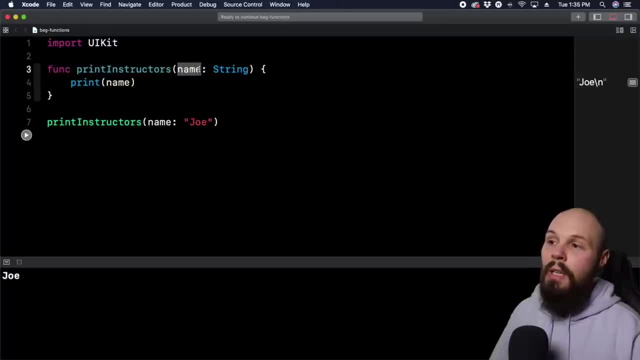 And then again down here in the scope. So this parameter label Joe gets used within the scope of the function. So within the scope of this function we have it here. So name is going to equal whatever we pass in, As you can see. 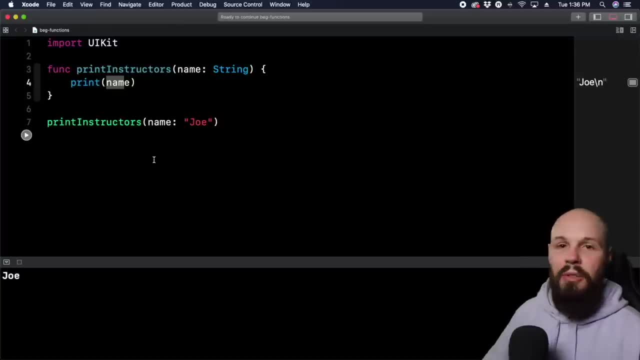 it prints Joe. So we're printing stuff and that's all fine and good, to just illustrate the point. but let's use an actual kind of real situation, because oftentimes you're not just going to print stuff, You're going to need neat things. 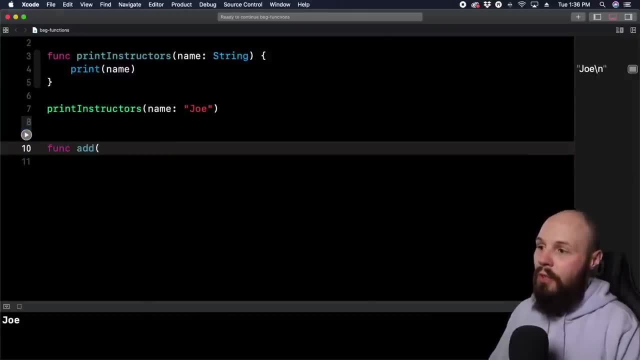 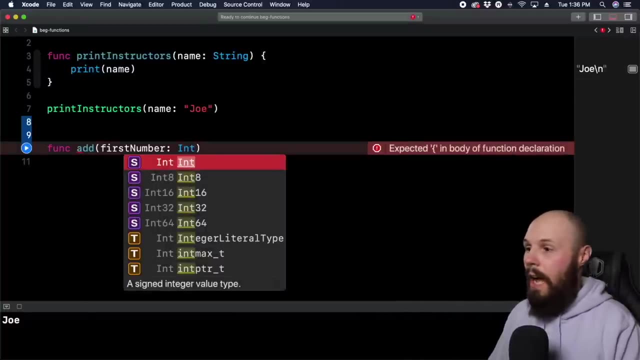 So let's create another function called add, and then we're going to do first number And then that is an int. Remember, every parameter you have to give a type. So we're going to add two ints together. So add first number, int. 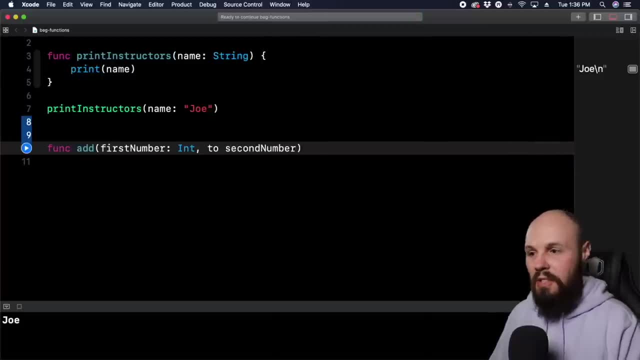 And then we're going to do first number int And then we're going to do first number int And then we're going to go to second number. Let's talk about this in a second. So second number is int in here. that is going to return. 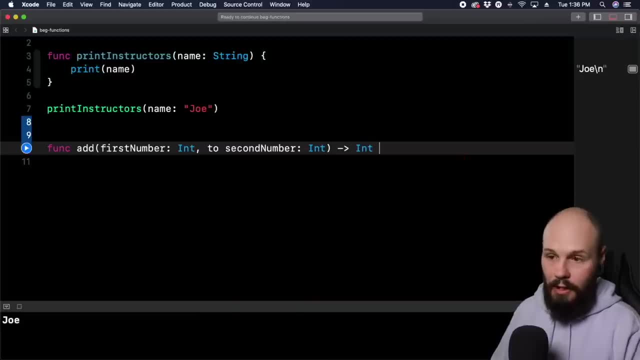 So this arrow means is going to return Something, is going to return an int, And let me explain that. And then we do open and closed. So let me run through this function: signature. That's what this is called, by the way. 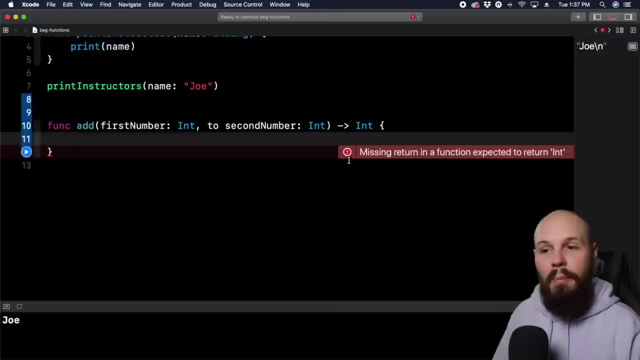 this is called a function signature And you see X codes yelling at me. I'm missing a return in a function expected to return an int. So what return means is it's going to do calculations and it's going to spit out a value. 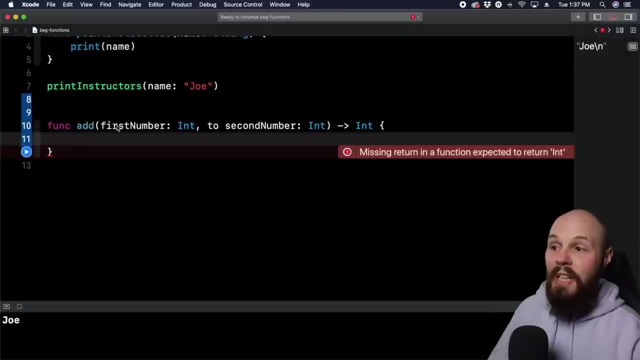 right. So you can kind of see what's going on here. We're going to: we're going to pass in a first number, pass in a second number, We're going to write code to add them together And then we're going to spit out the value. 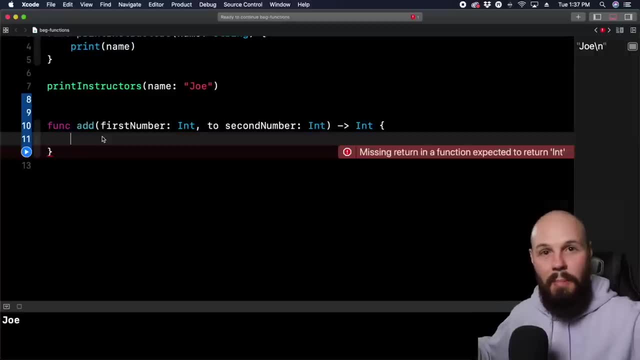 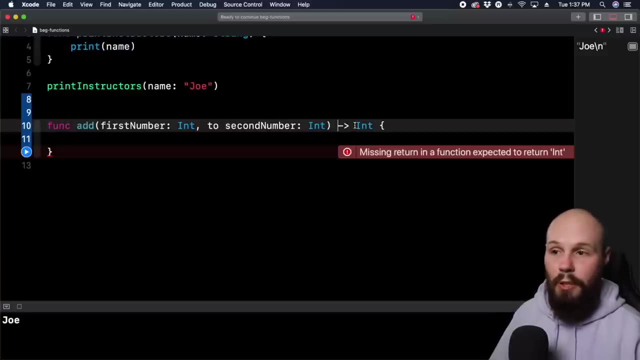 This is kind of like a little factory, right, It takes in two numbers, spits out the sum. So when you want a function to return, you create this arrow, which is the hyphen, and then a greater than sign, And then you have to give it a type that you're going to return. 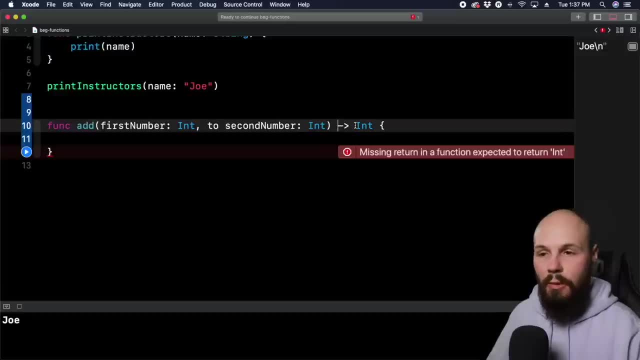 right, Like I can't return a string here because an int plus an int is not going to equal a string, And what X code is telling me again is that I don't have the return function, So it's just letting me know that I have to specify that. 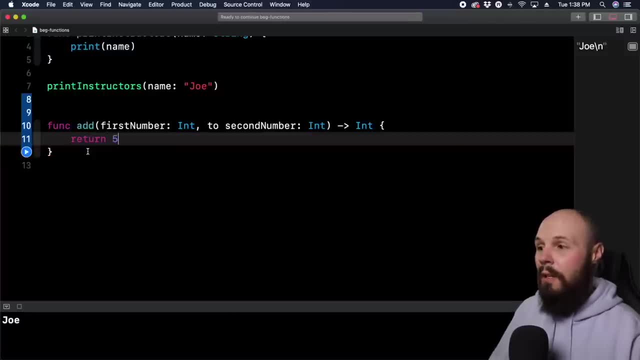 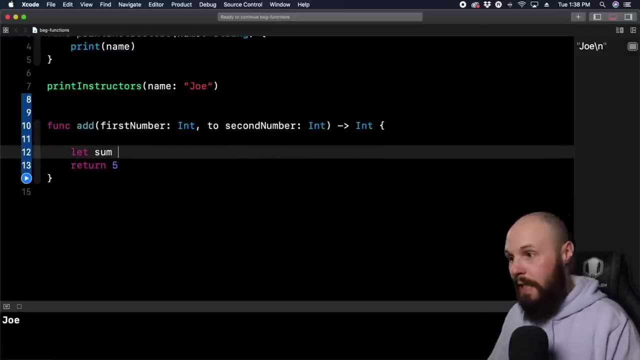 Hey, I'm returning something, So I'm going to return five right now just to get rid of the air. We're not actually going to return five because we got to do some math first. So in here what we can do is let some equals first number, because I'm passing in a 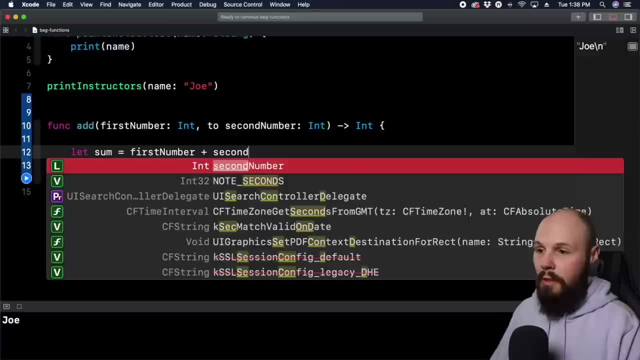 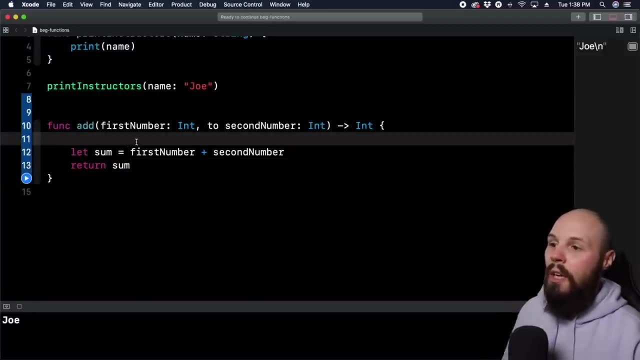 number plus second number. And then we want to return the sum. right, We want to spit out the sum outside of our factory here. Now let me talk about this too. right here, This is called an argument label. This helps your function be more readable. 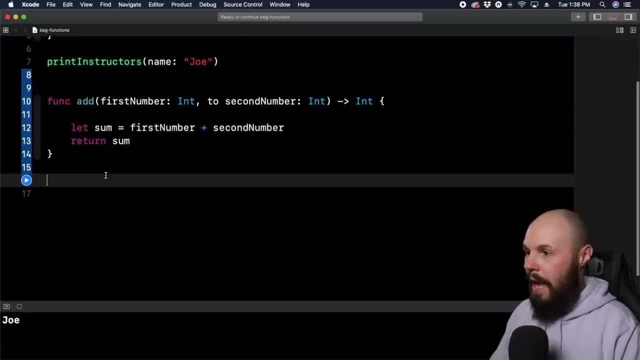 Let me show you. So now, when I call this function down here, I can do add, and you can see first number to second number, So it just reads nicely. So if I wanted to add 18 to you know one, 26,. 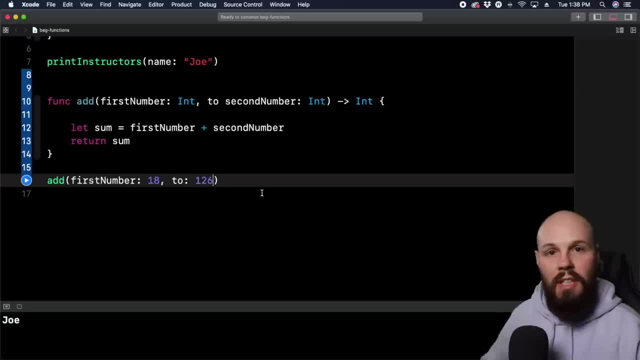 right. Add a first number, 18, to one, 26.. It's more readable And that's the benefit of Swift, is it's? it's very, it's nice to read, right? If you've seen other languages, it can be brutal. 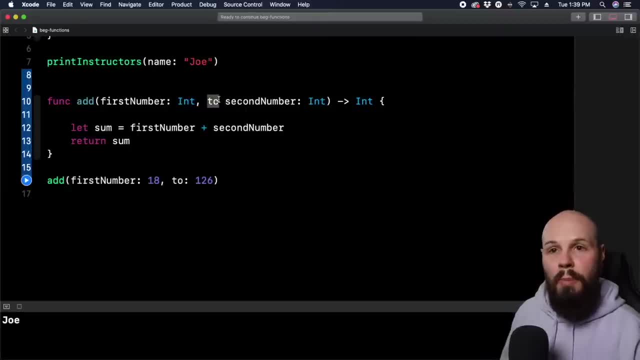 And what that did up here was the argument label is what shows up. This is called the call site wherever you use your function. right, Remember, you define your functions logic and then you have to use your function wherever you use your function. 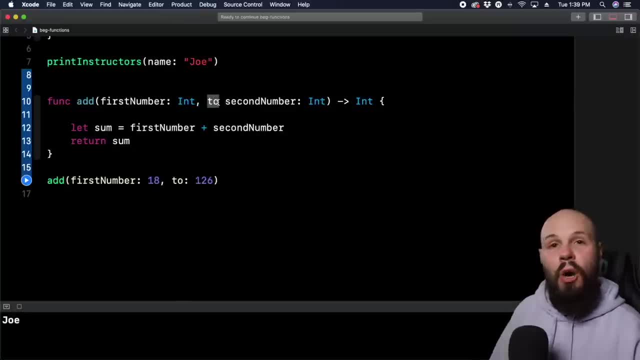 It's called the call site. So what your argument label does is helps your call site be more readable. So again, argument label gets used at the call site. This is the parameter label. The parameter label gets used within the scope, right. 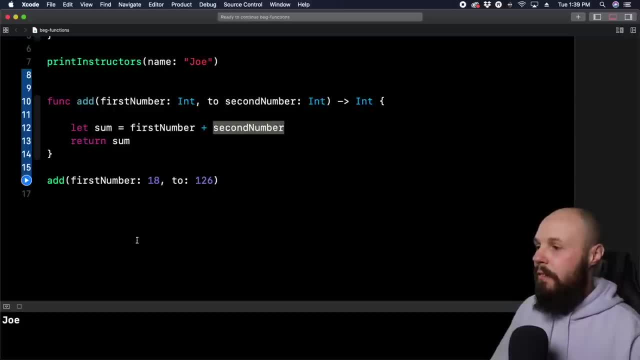 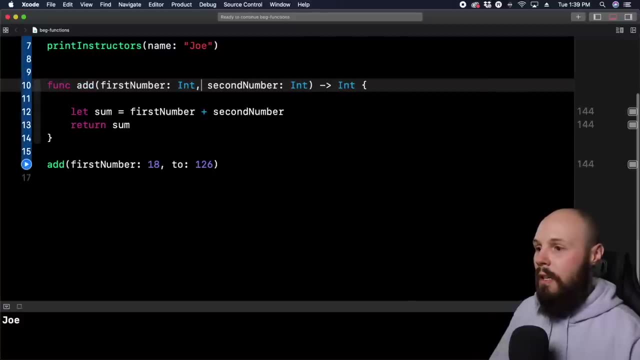 So that's why we use second number down here, And if I run this we should see yep one 44 over here on the right. Let me just kind of illustrate that. Let's get rid of this argument label, And this one won't read too bad. 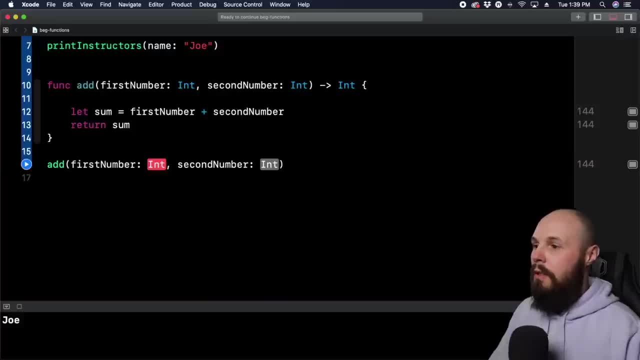 But you can see, add first number. you know 14,, 100, right. Add first number, second number. It doesn't read as well as add first number two and then a number, right? So again, this makes sense. 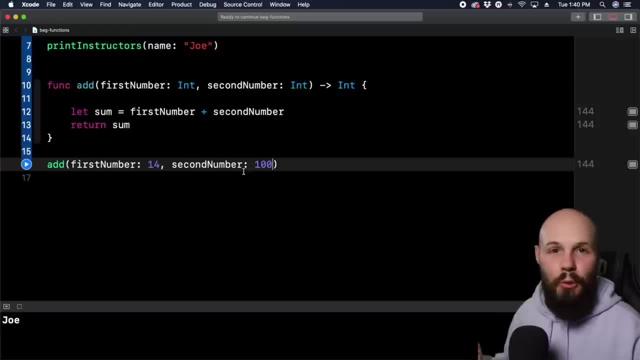 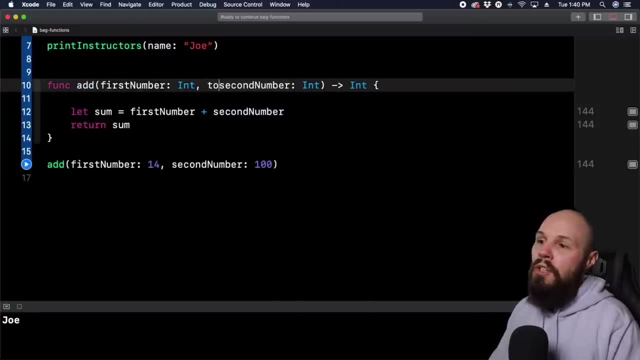 but it's not as human readable, And in Swift you strive for that human readability in your code. Trust me, when you read a code base that reads nicely, you're really going to appreciate it. So anytime you see two words up here, 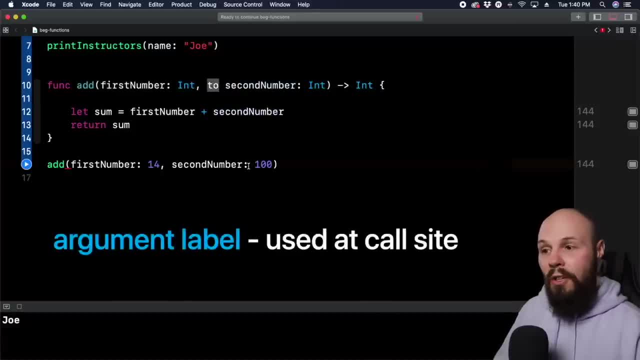 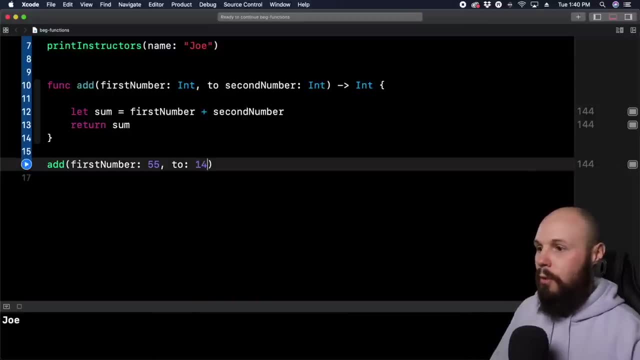 remember. the first one is the argument label which gets used at the call site. Let me get rid of this here. Okay, Add first number two, Yep, You know 55, two one, 14.. So the argument label gets used at the call site. 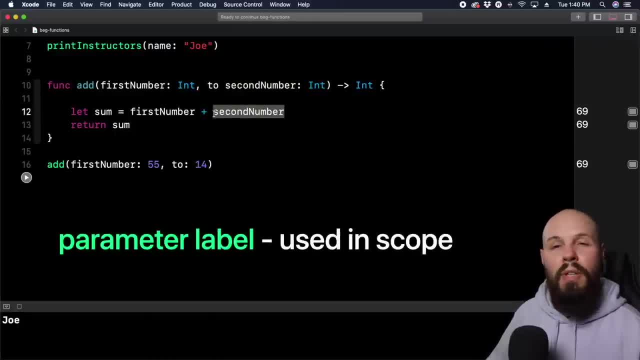 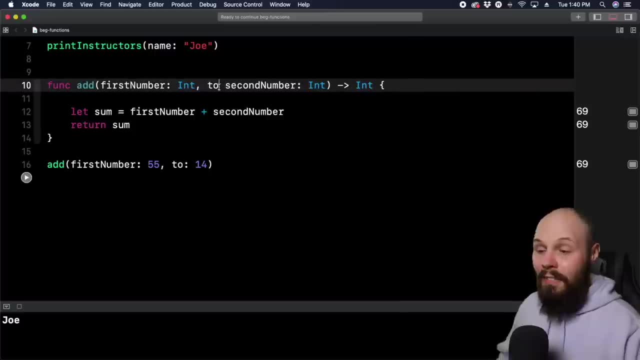 The parameter label, which is the second one, gets used within the scope. I know this is very confusing for beginners starting out. They'll see multiple like labels up here. They don't know what that label means. And again, I could have named this anything I want. 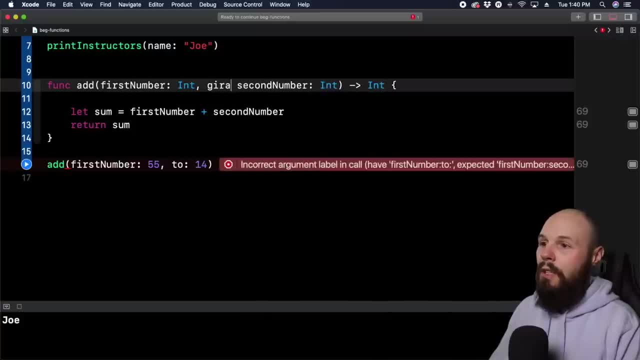 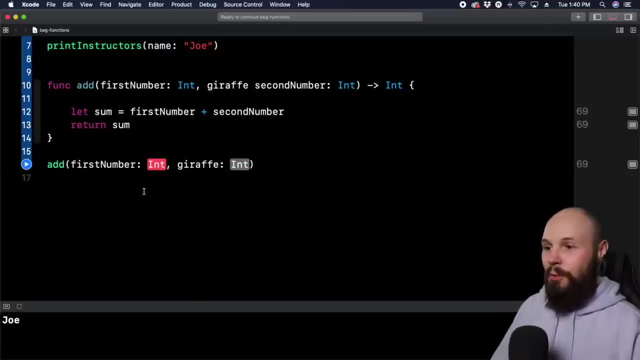 I could have named this like a giraffe right, If I wanted to. And then now here at the call site I'm going to get add first number in giraffe int. Obviously that makes no sense, but I'm just illustrating that it doesn't have to be like two. 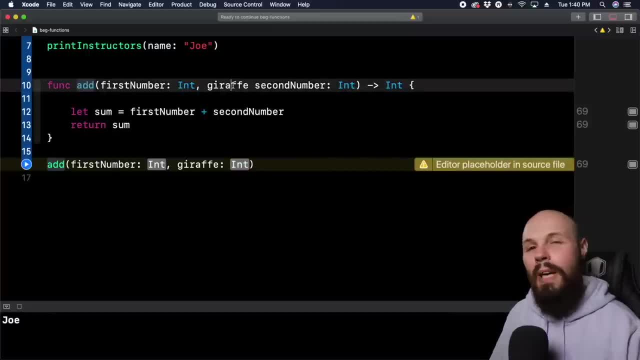 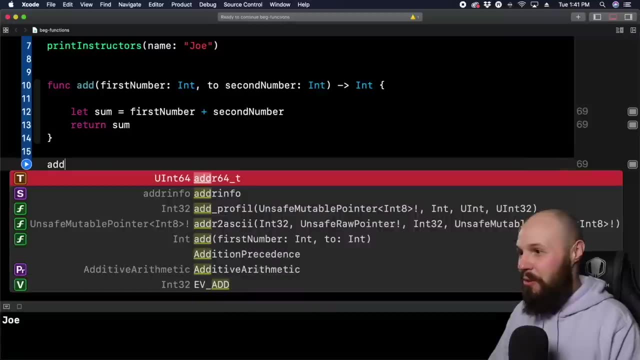 four or on, cause that's often what they are, but they can be whatever you want to name them, So it makes sense. All right, let's go back to two here. I don't want to. I don't want to use ridiculous examples to confuse you too much. 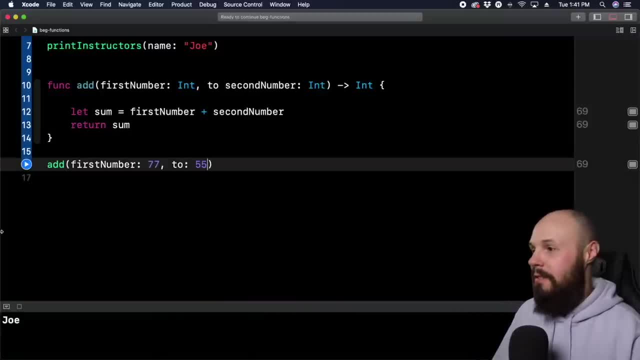 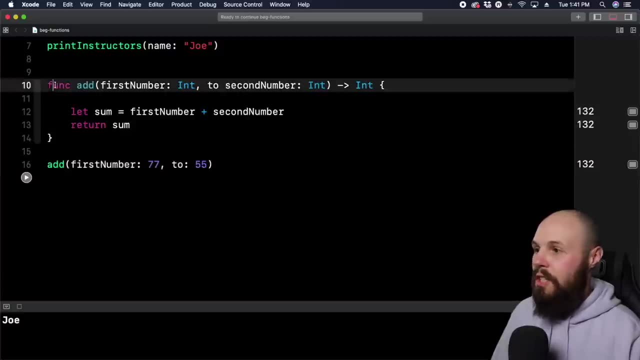 but hopefully that drove the point home. 77 to 55, right Run it so you can see. let's run through this function again, just to show you all the parts to again really drive the point home. function add. That's the function. 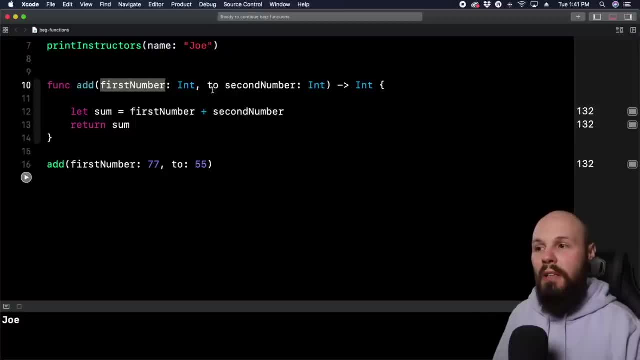 Name. Our first parameter is first number And you may notice that, like this, this one only has one label. by this one has two. by default, your parameter name will be used as your argument label at the call site If you don't explicitly use one, like right here. 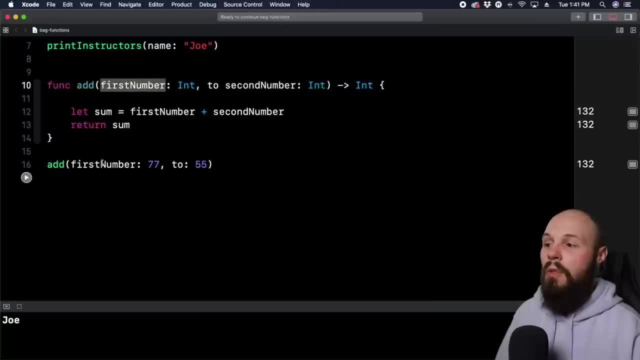 we're using two, So that's why it shows up. but we didn't use an argument label, So the parameter name shows up down here at the call site. But anyway, a parameter label you have to pass in a type. Remember we're adding two ends together. 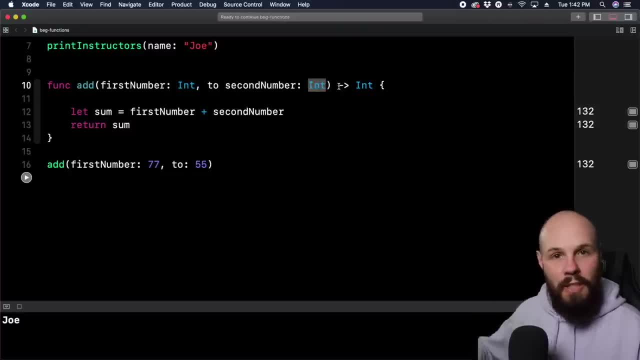 passing in another type for the second parameter, And then we're returning Cause again. remember, this is a factory. It's taking in two numbers, spitting out another number. This is returning is what it spits out. It returns an int. 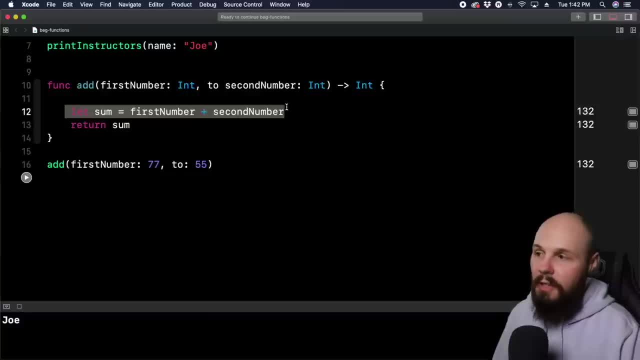 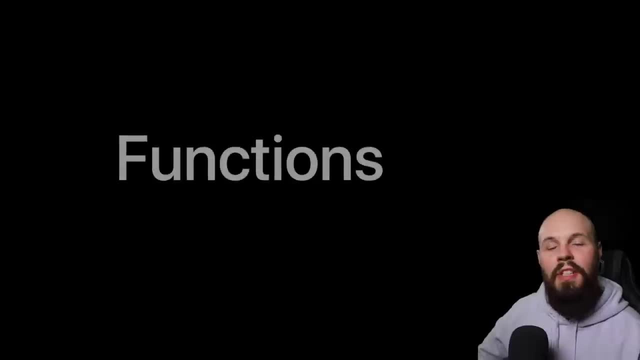 So you can see, here's where we do our basic arithmetic: first number plus second number, and then you have to return the sum. So, again, this is you actually spitting out what you want to spit out of this function. And let me finish this video by showing you a relatively complex function. 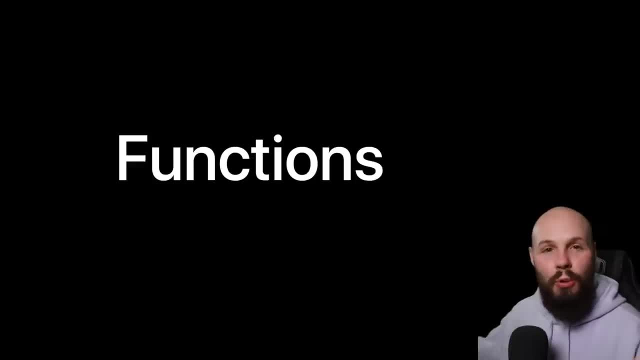 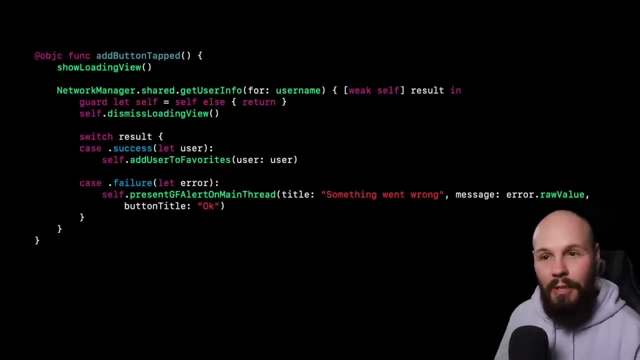 Again, I do not expect you to get this, but I want to show you kind of what it's like in the real world and how you can use functions inside of functions. So here on the screen, this is what happens When you actually tap the add button. 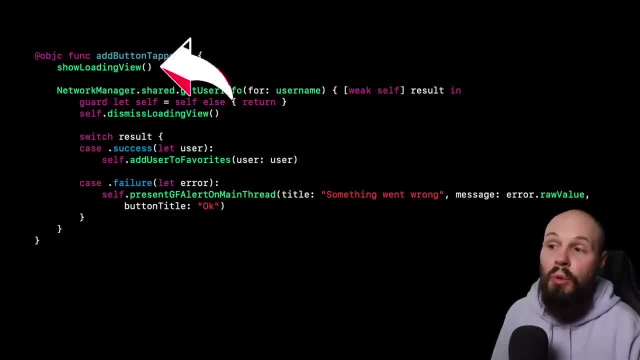 right, We're adding a user to the favorites So you can see we're calling show loading view. That is another function, So you can use functions inside of functions. right Cause when we add button tap we want to show the loading view and then we're getting the. 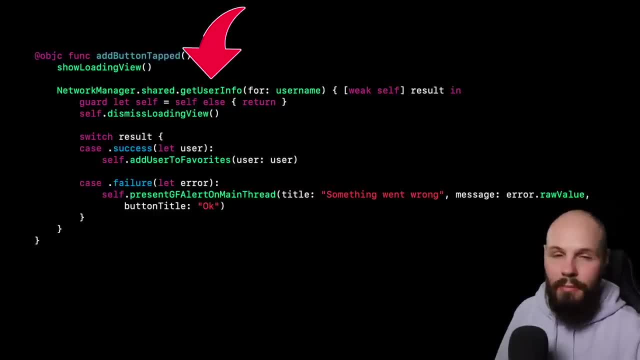 user's info. This is a network call. This is hitting up a server downloading the information again. don't worry about that, but you can see. then we dismiss loading view, which is another function, And then we're using a switch statement on results. more on that. 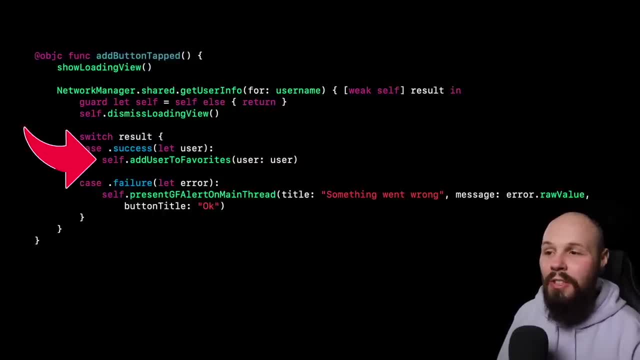 in a bit which has more functions in it. you know, add user to favorites. You know, present alert on main thread. That's another function. So again, don't be intimidated by this. I just kind of wanted to show it to you, like in. 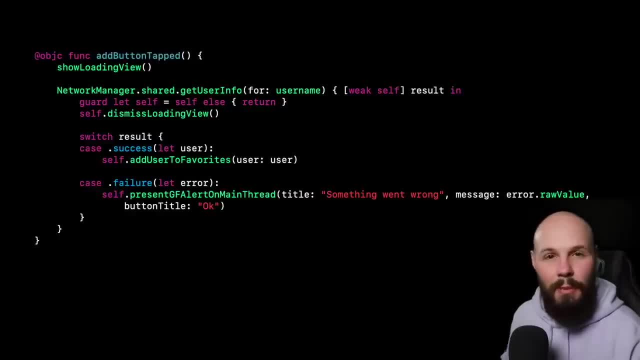 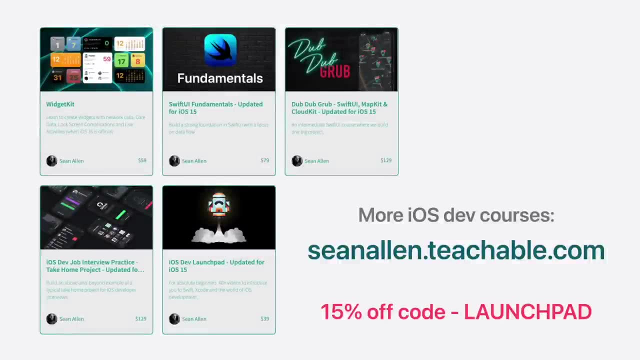 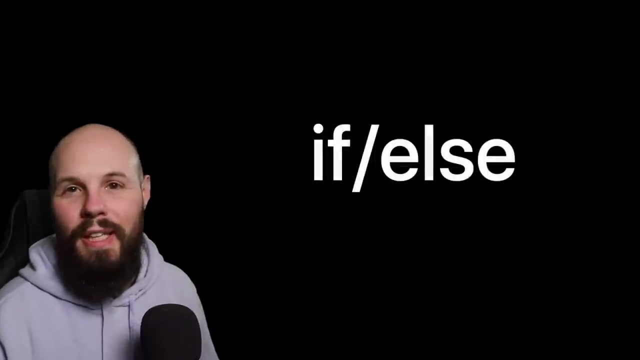 action in the real world. So you have an idea of how all this can come together. again, don't be intimidated. But anyway, onto the next video, onto another very important and very common thing, And that is the if else statement, and this is basic logic that almost all computers use. 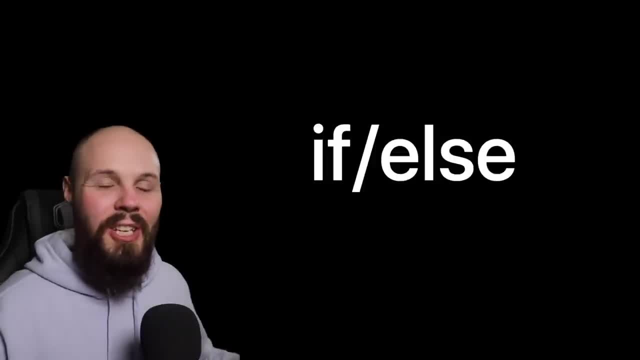 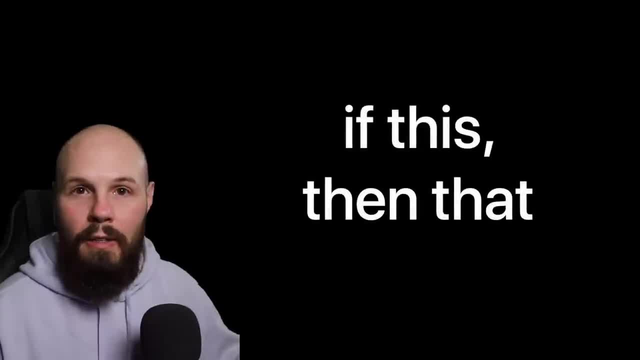 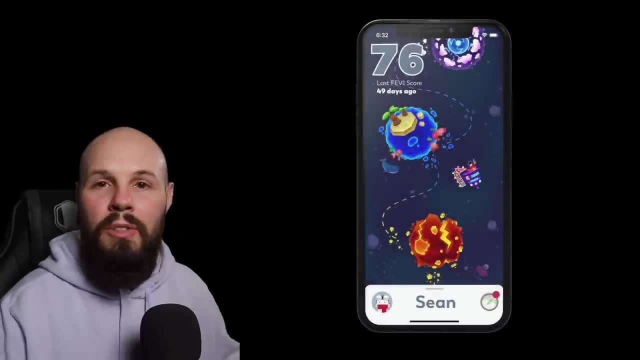 It's a simple statement that says: if this happens, do that or do this. Right. It's just the basic logic, You know. if user is logged in, send them to the home screen, else, send them to the login screen. 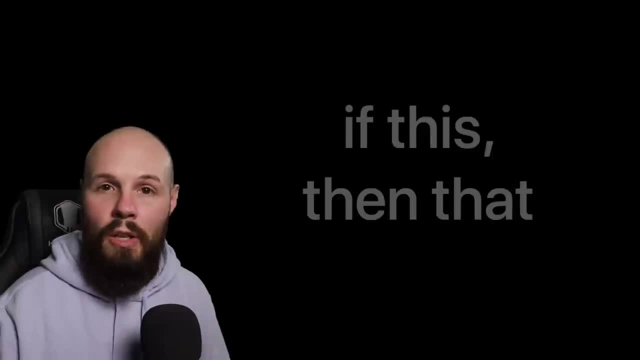 right. So if they're not logged in, they go to the login screen. If they are logged in, they go to the home screen. So again, it's a basic: if this, then that. So let's dive into some code to create our example. 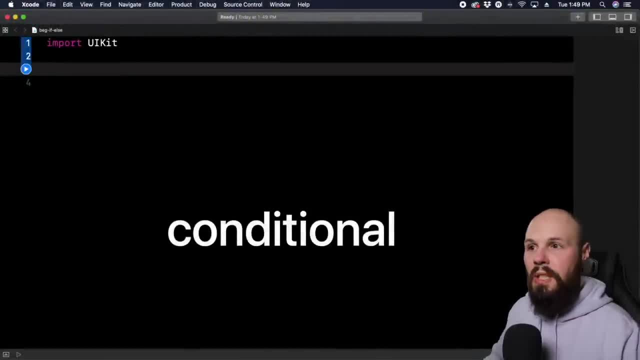 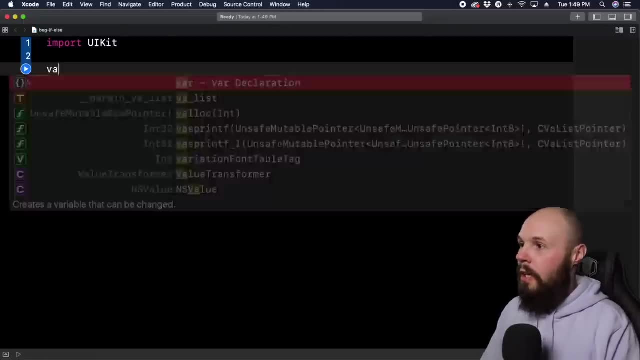 Now, if statements are based on what's called a conditional, okay, Conditional is something that is either true or false. Let's create our conditional right now, So it's gonna be a boolean. Hopefully you put that together. So var is dark mode on. 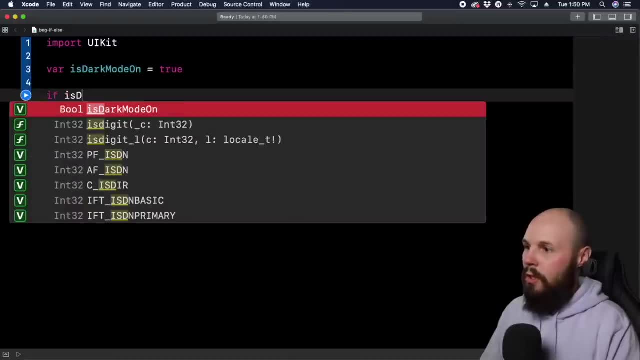 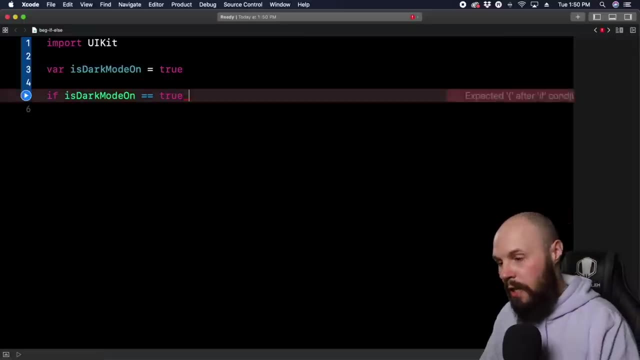 equals true. So if is dark mode on equals equals true and actually don't have to type that, I'm just leaving it there so you can really see what's going on- and then we create the scope of our if statement with Our curly braces here now: equals equals. 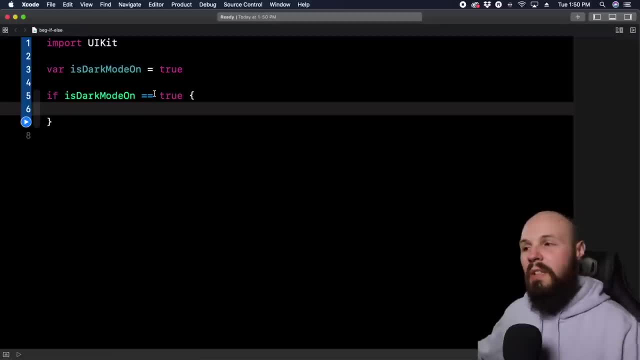 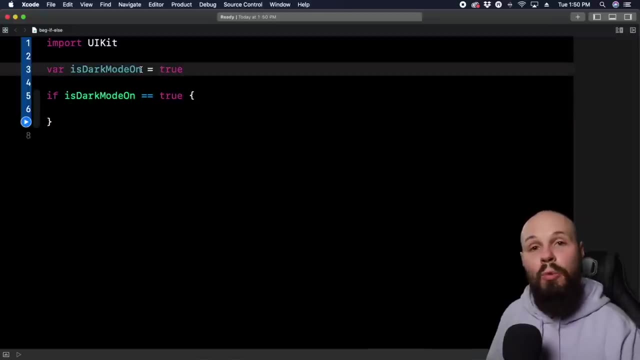 Means, is it equal to more on operators in a later video. but one equal sign mean we're setting the value right. So this equal sign means we're setting. is dark mode equal to true To equal science? means we're checking it like we're checking if dark mode on equals true. 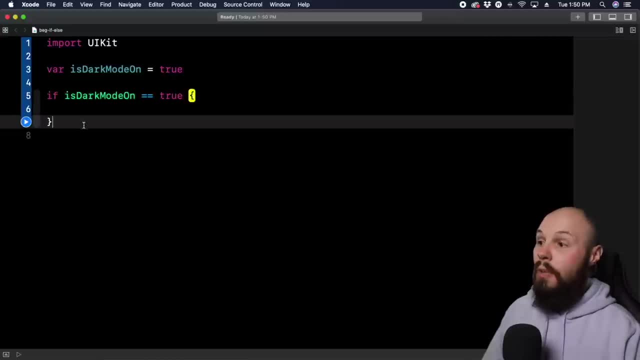 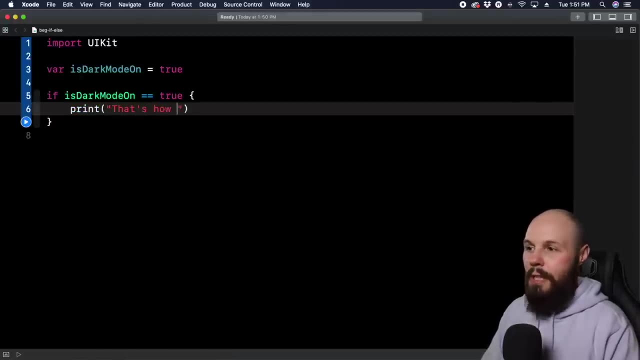 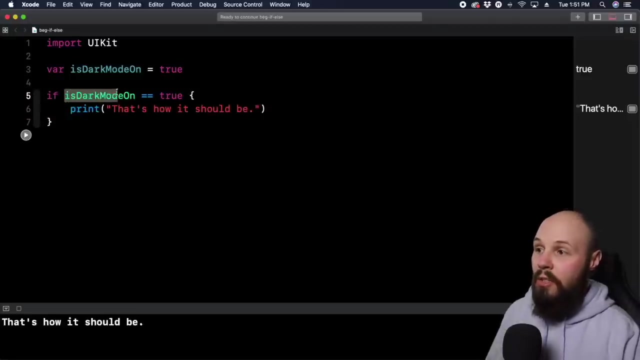 So again, more on the operators later, but that was a little sneak peek. So if is dark mode on equals true, then we want to print. That's how it should be right. so Now when I run this, it's gonna print that out because it's gonna evaluate, it's gonna check: is dark mode on equals true and up. 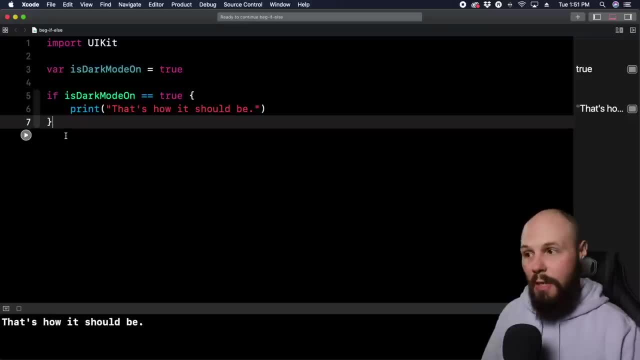 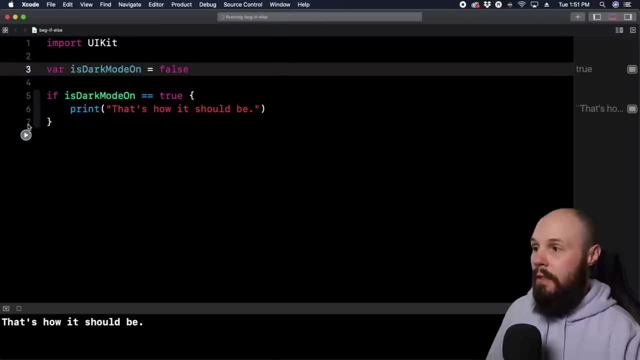 Here on line three, it is now. we don't have an else statement. So what's gonna happen if all you have is just the if is: if this checks out to be false, So let's make this false, Run it again. You'll see nothing happens. So what happens in this code is it goes down, it checks, is dark mode on and if it's false, it just continues on it. 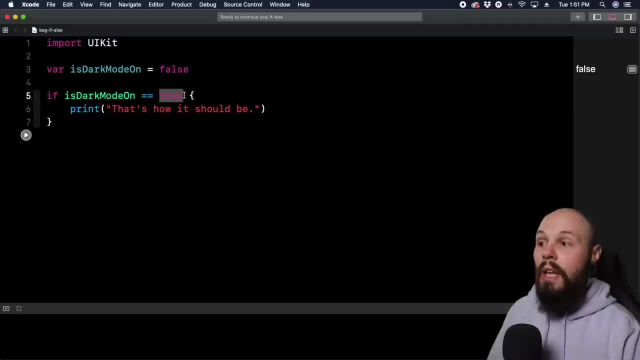 Doesn't go into this, into the scope here. if it's true, Then it goes into the scope and prints this out. So that's why, if I flip this back to true now, it's gonna go into that scope and it will print out. That's how it should be. 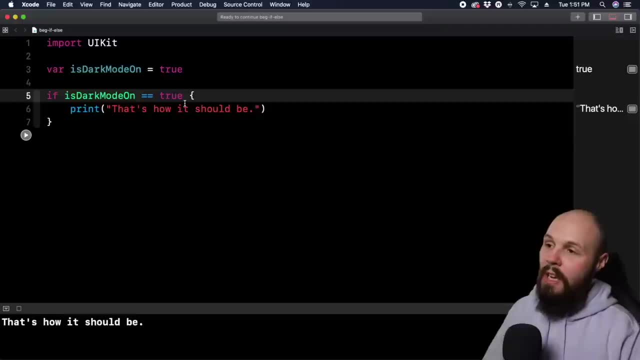 So there you go. Now, like I was saying is, I don't have to type this. Xcode is smart enough to. if you have a boolean like that, It defaults to true, like a defaults the first check to be true. But I wanted to type that out so you could actually see what's going on. 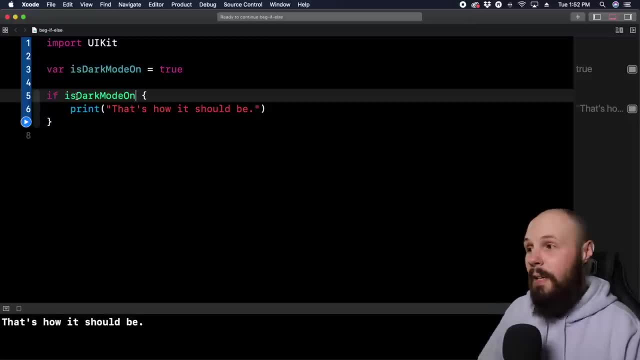 But from here on out we'll just do: is dark mode on, because again it reads better, right, if is dark mode on? and that's Why you title your booleans again. This is all just like best practice and convention. That's why you want to tell you your boolean something like that. 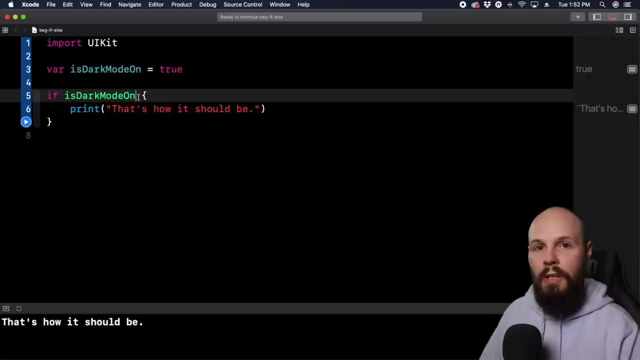 Like: is dark mode on, is user logged in, etc. So that's the very basic level of in this statement. But now let's add the case where we want to do something different if dark mode is false. So that's where you do else and then give you another scope. now We want to print. 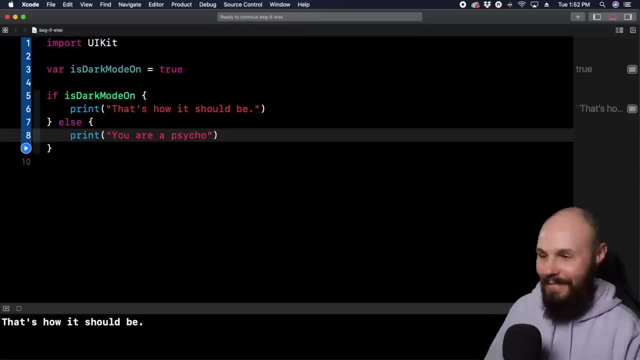 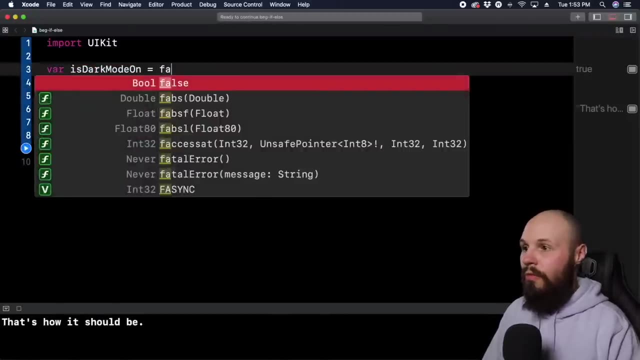 You are a Psycho. Just kidding, Not really, Anyway. so now let's run it. dark mode is true, So we're still gonna get. that's how it should be. now, if I flip dark mode to false, It's gonna go into the else statement and print: you are a psycho. 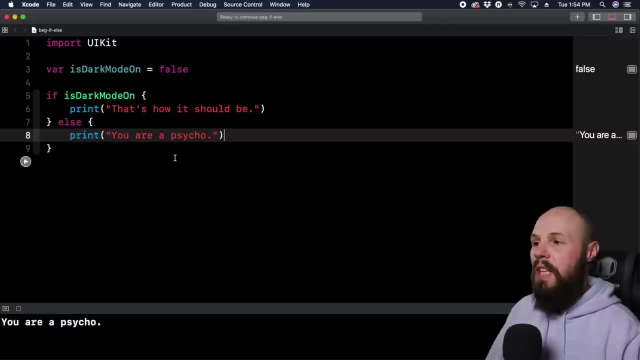 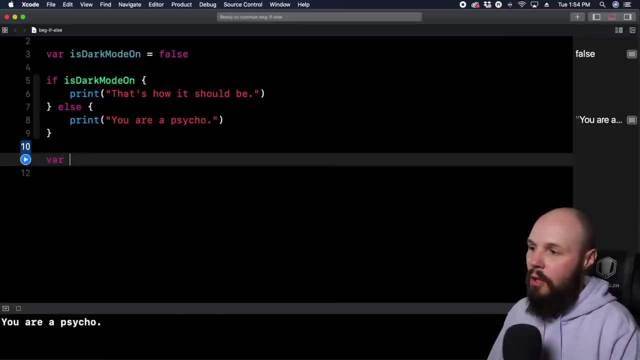 There you go, should you dark mode? So that's the basic if-else statement, based on a very specific boolean that we already have, But it doesn't always have to be a specific boolean. Let's say: let's do something real quick, So var. my high score equals five, five, five. 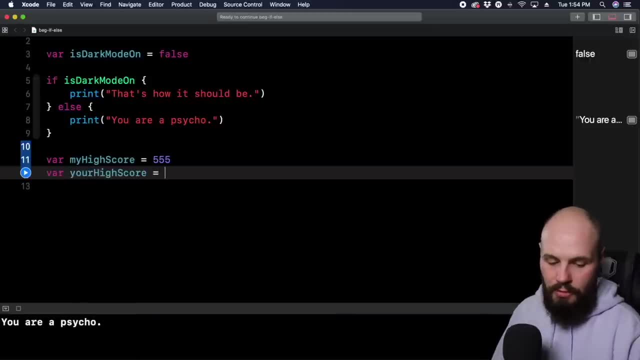 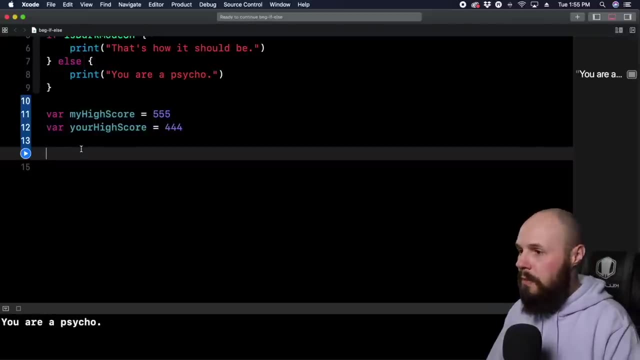 Var, your high score equals, you know, four, four, four. right, Those are your scores. you can do again. It just has to evaluate to true or false. again, That's the conditional. so you can do if my high score is greater than your. 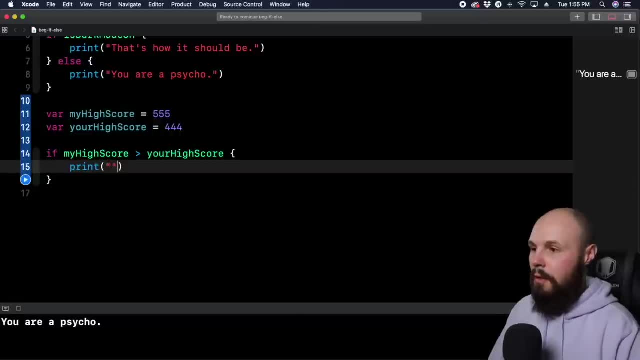 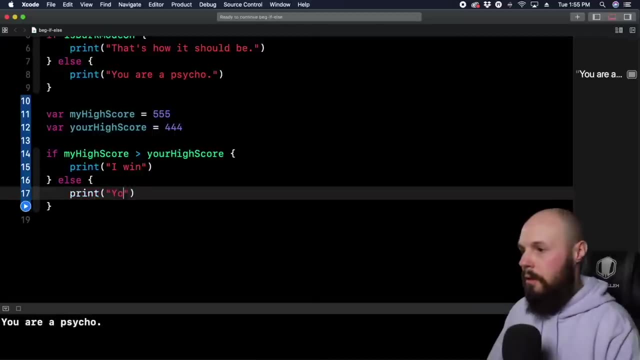 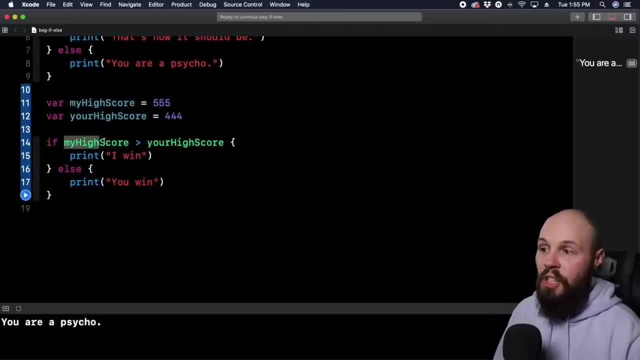 high score. Let's print I Win, else print You win. so you can see I don't have like a specific is dark mode on boolean. here I kind of created my own just to check. you know whose high score is higher, right, So mine is higher right now. 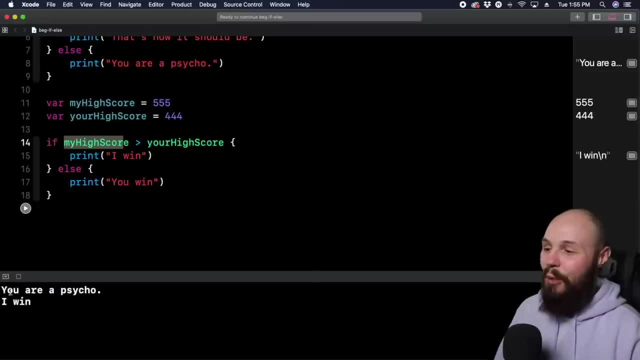 So I'm gonna print. that's funny, I didn't even mean to do that. You are a psycho, I win. Yeah, anyway, that made me laugh and you can see if I make mine lower. Do one, one, one. you're still gonna be a psycho, but you're gonna win. your psycho, you win. Let's actually. 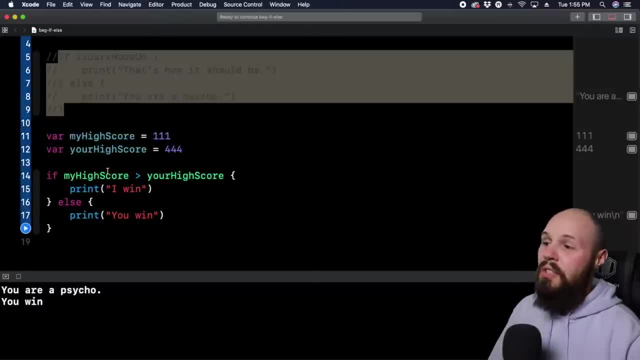 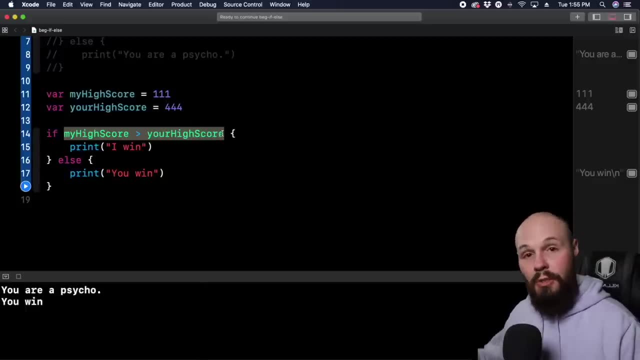 Comment this out. It's kind of funny So you can see. the main point I wanted to show there was: it doesn't have to be a specific boolean, Anything that evaluates to true or false. again, if something is greater than or less than, that's gonna be true or false. 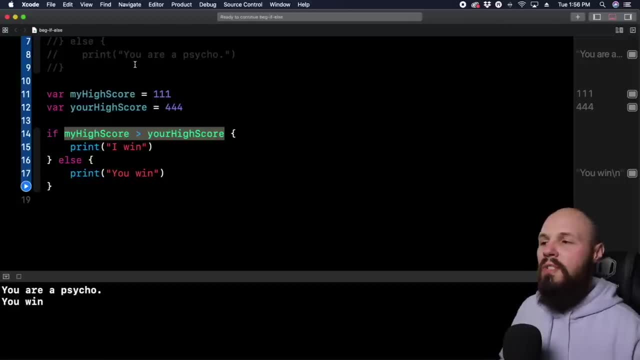 You can use that as the conditional in your if statement. now we've covered the if statement. if there's only two paths- right, True or false- Well, what if there's multiple paths? Let's take, let's change this back to high score. 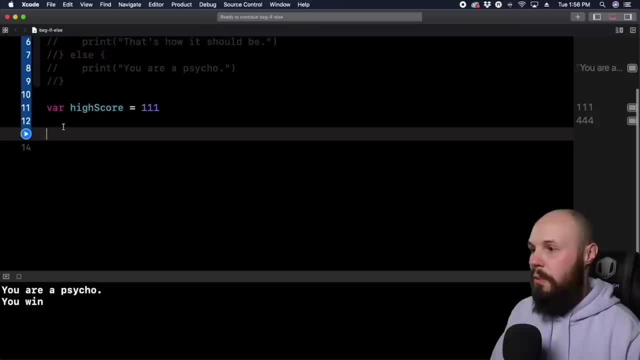 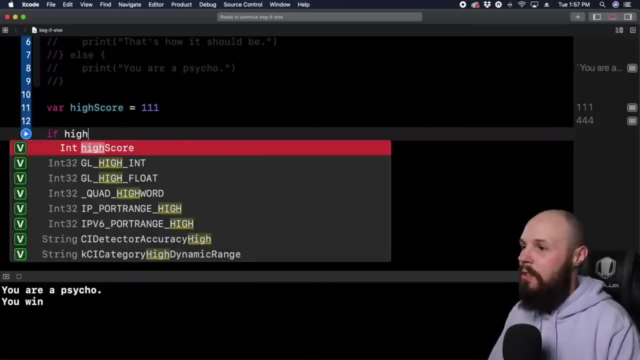 And let's get rid of this and we can start over from here. So we just have a high score, so we can check multiple paths. Like, let's say, we want different levels to this right. For example, if high score is greater than 500, We want to print. 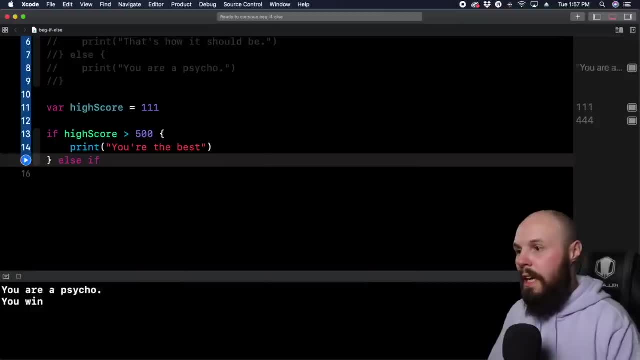 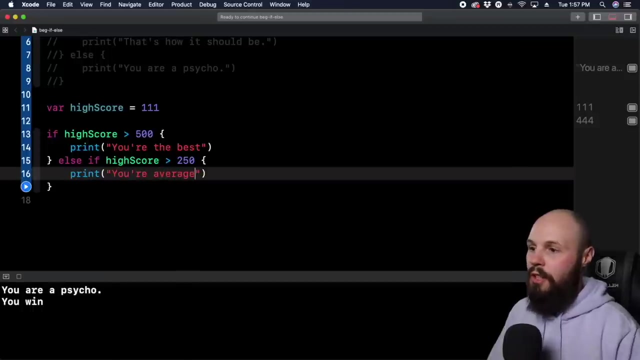 You're the best. and then we do else if- and we can do else if, if you have multiple paths. And this is where you put the next conditional: else if high score greater than 250 print. You know your average. and Then the final one: we can do multiple else ifs. we can do else if high. 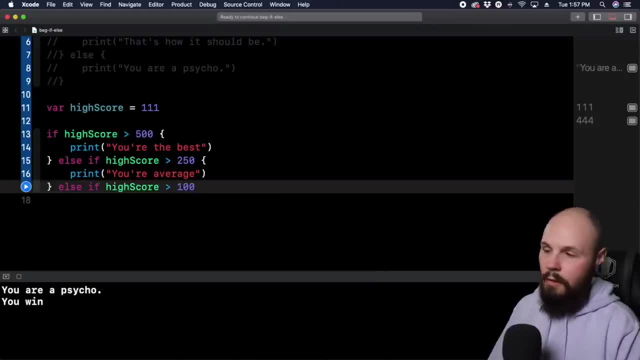 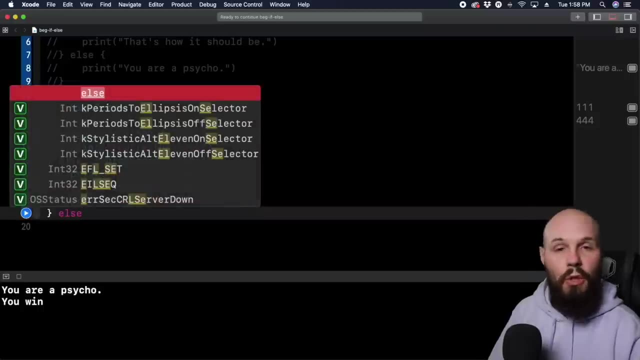 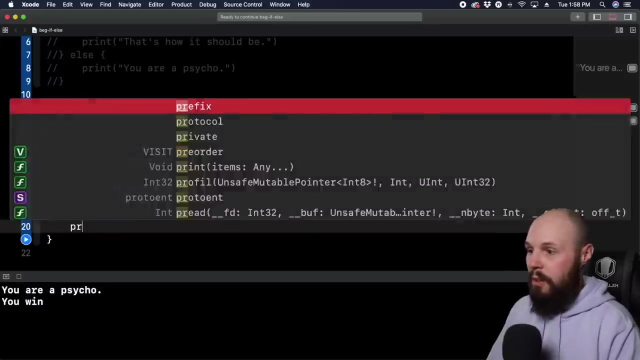 score greater than you know, 100, Print. You need improvement and then else is always the final one. You don't need else if for the final one, so else kind of catches all the other cases. So basically anything less than a hundred we're just gonna print, You know. 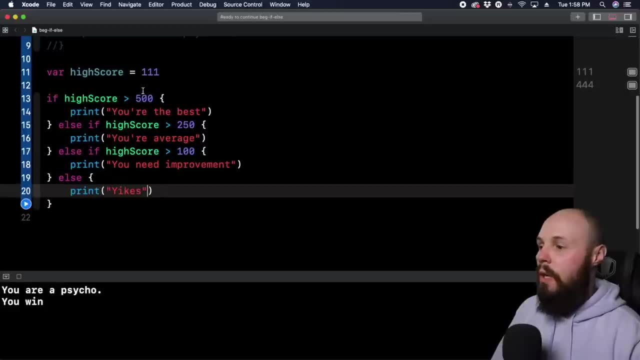 Yikes. so you can see there's multiple paths that we're going here, So let's run it. So what is our high score of 111? get us, you need improvement. So how this evaluates, right, it checks first. it says: is the high score greater than 500?? 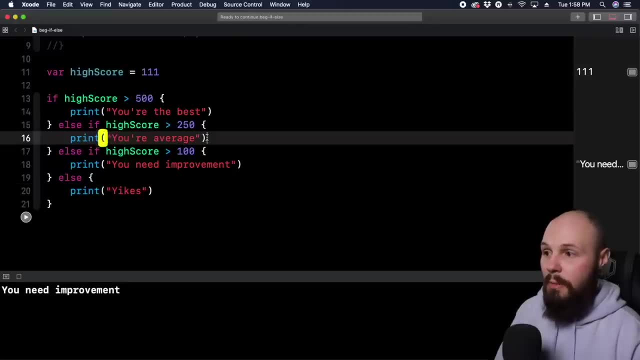 Well, the answer is no, so then it goes into this. next else if statement- and then it checks again- It's high score greater than 250. No, so then it keeps falling down until it finds one that is true. So else if high score is greater than 100. Yep, That's the one. 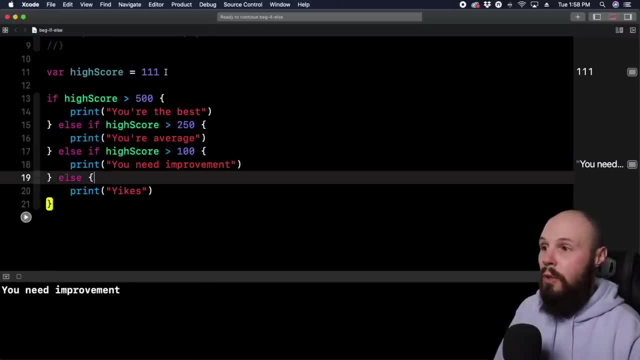 Then it goes into here and prints: you need improvement. So let's try another one. Just give me my high score of a thousand. Well, again, it's going to check this first one. Oh, we're greater than a thousand. Okay, we're done. go in here, print. 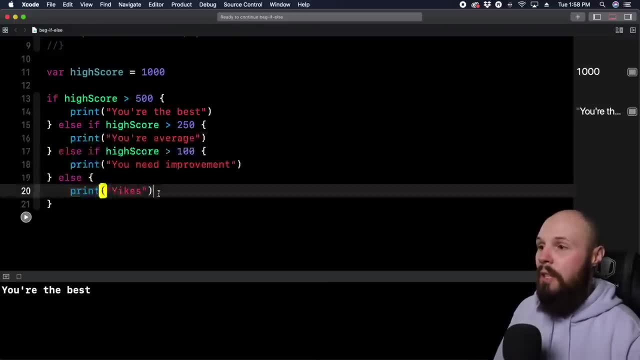 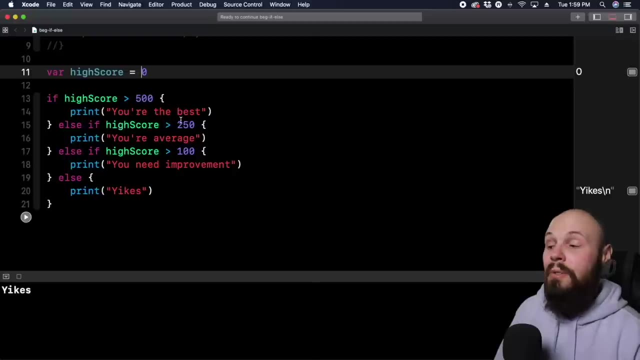 You're the best and we're done. We're not gonna evaluate anything else. Give me a big fat zero. here And again. it's gonna go through all these. it's not greater than 500. It's not greater than 250.. It's not greater than 100. 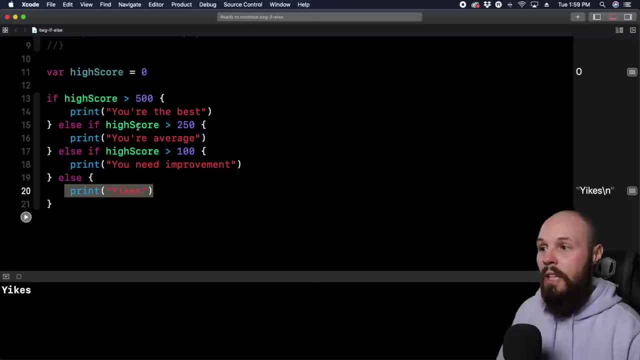 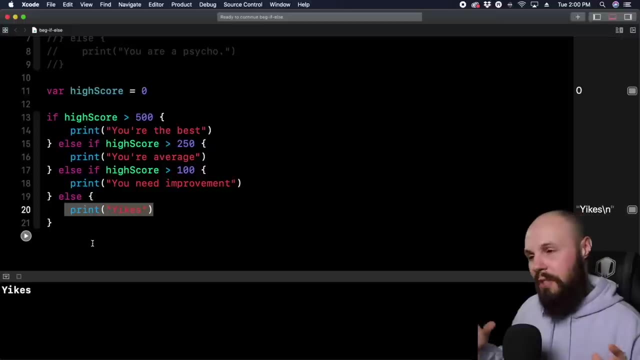 So it falls into this else statement Which again is kind of like that, the catch-all, if none of these equal, true, And then we just print yikes. So those are some basic if statements. again, that is foundational knowledge You're gonna use if statements all over the place. So hopefully you understood it. And again, it's basically if this, then that. 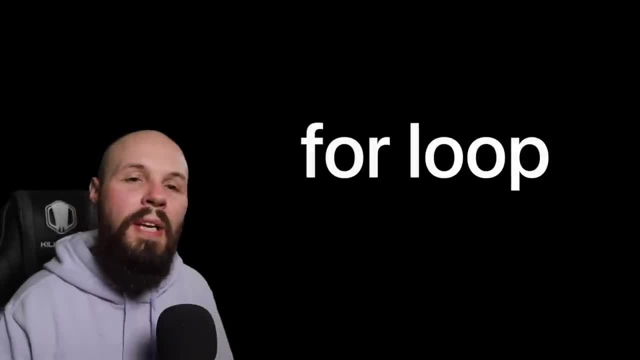 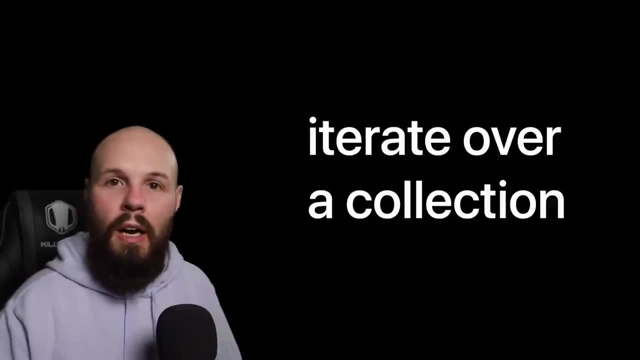 All right, Let's talk about the basic for loop, and there's really two very common ways that you use them. One is the iterate over a collection number- a collection is like an array, a set, a dictionary, And another is to do something a certain number of times. now, 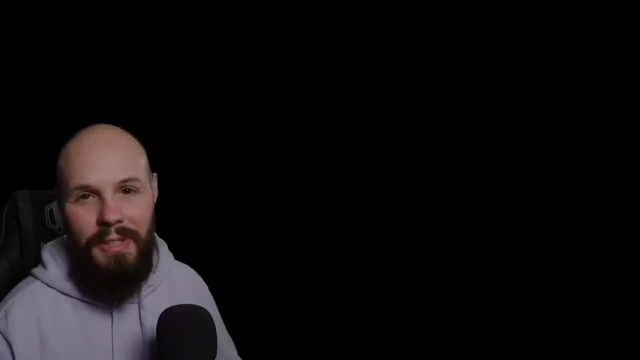 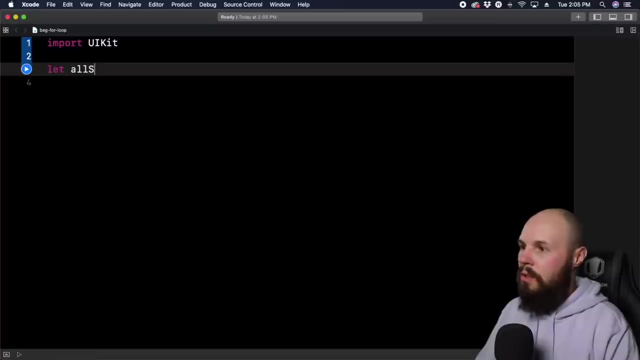 The best way to explain that is to actually show you. so let's dive in. So to use our for loop, the first way of iterating over a collection. We need a collection, So let's create an array, let all stars Equal, and this is going to be the the LeBron's team all-stars from this year game. So LeBron James is the first one. 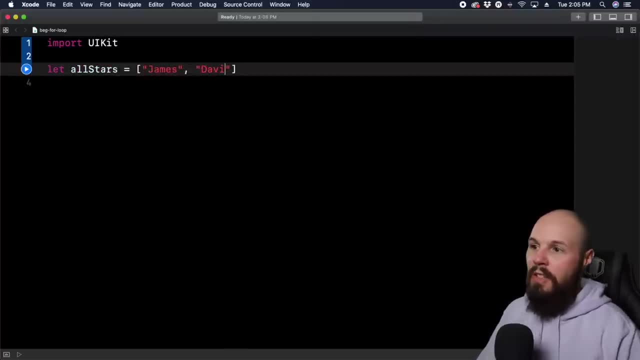 I'm just gonna use the last names here as well. So Davis for Anthony Davis and Harden and Donchik do and CIC, and Who is the? Leonard Kawhi Leonard. So again, that's the starting five for LeBron side of the NBA all-star team, if you don't have that context. and it's just their last names. 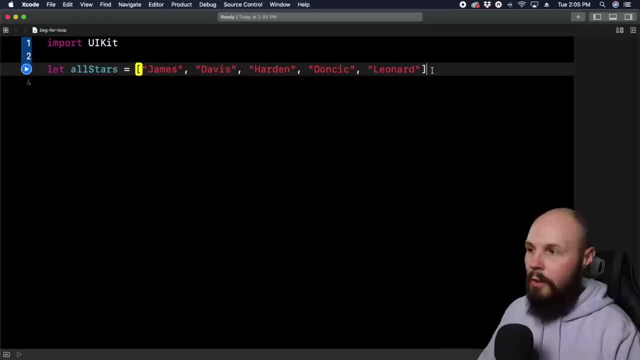 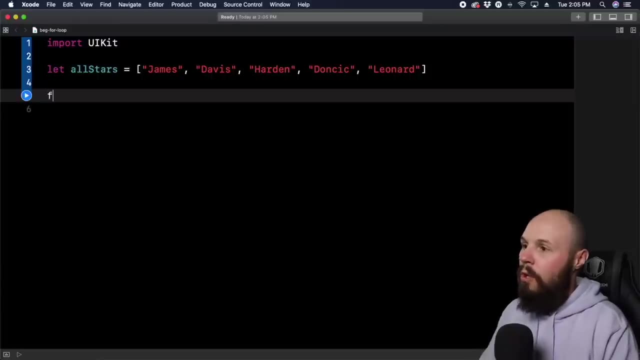 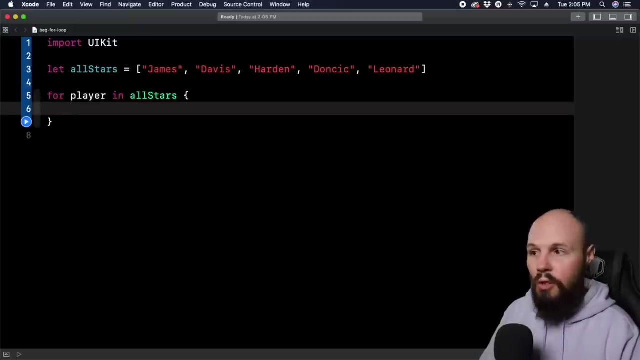 So this is our collection that we're going to use to iterate over. So here's how you write a for loop. It's best for me to actually write it out and then I'll explain it. So for player in All stars. and then here's the scope: right, the open and close curly braces creates our scope. 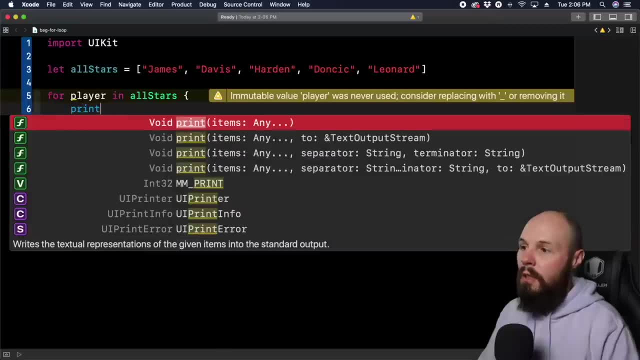 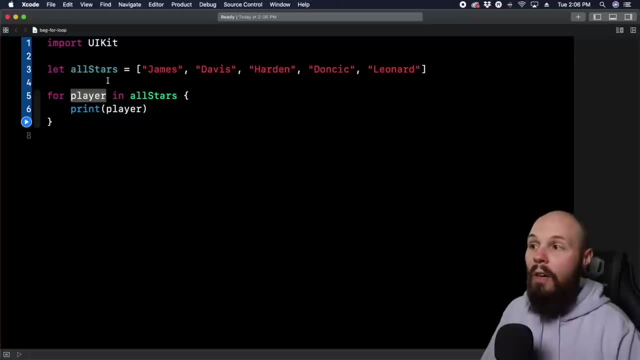 So what do we want to do? And there is: we want to print Player. now, let me explain this before I run it. So what this is saying is: for every player in the all-stars array, I want to print their name. That's what it's saying. 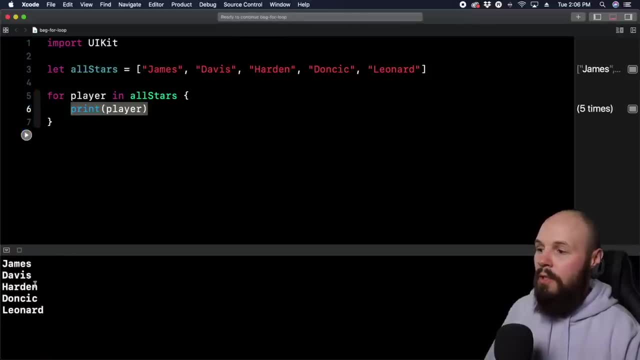 So if I run this again, you can see we print it out: James Davis, Harden, Donchik, Leonard. again, It printed out in the order because, remember, arrays are ordered, that They're in Now this player can be anything I want. right, I named it player because that makes the most sense. and again back to 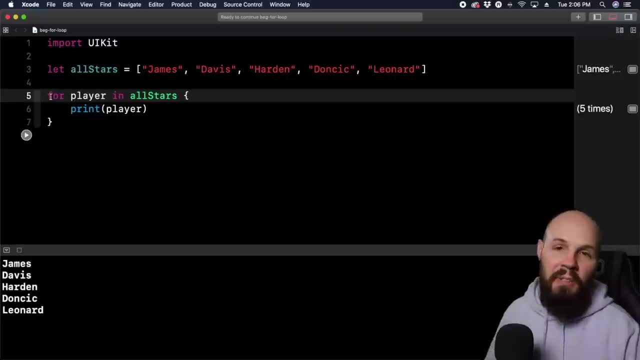 Being readable the way you write your code. you say for player in all-stars, like kind of makes sense, right? You may also see a lot of people do like for item in, you know, And whatever the name of the array is, and then you know you want to print each item. 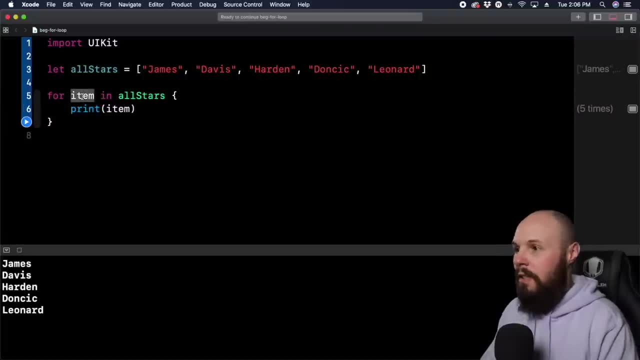 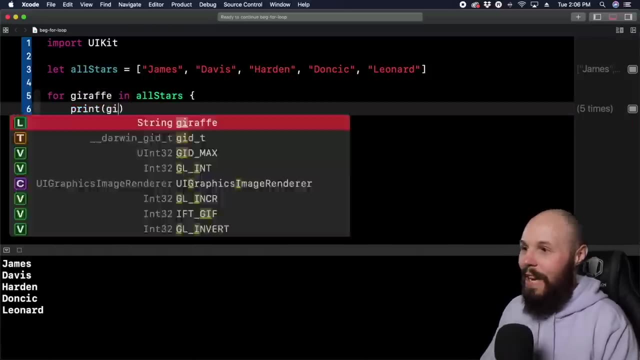 That's fine, But item is generic. Like I said, I think player makes more sense, but you could again. if you wanted to call this a giraffe, You could. I don't know why I keep going back to this giraffe example, But my point is because I know I've gotten a lot of confusion before from other beginners. is they thought this had to be named something? 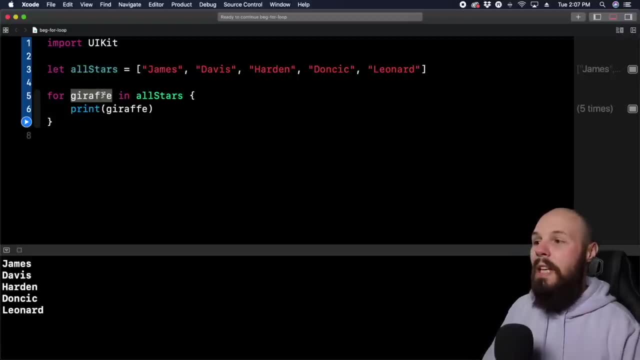 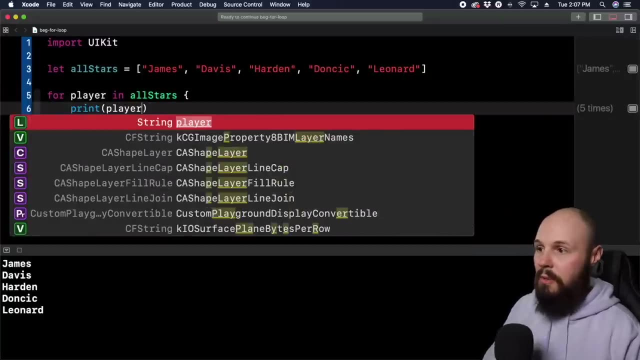 specifically, and I want to really emphasize that this needs to be named whatever you want to name it. So it makes the most sense for your code base and in this code base, Player makes the most sense. So, again, for whatever you, whatever item, and then this is every item. 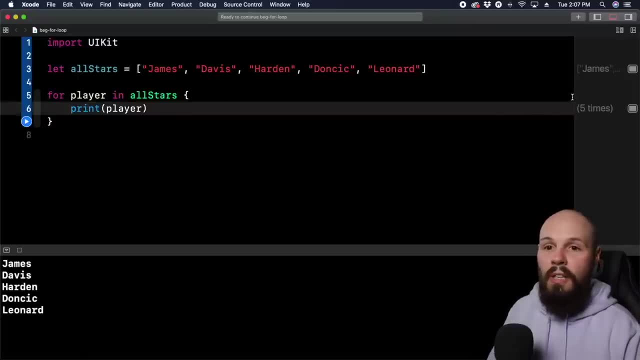 So right. so what happens is is: this executes, as you can see over here, Five times. So that's the beauty of playgrounds: It'll tell you how many times it executes. so what happens is The first time it goes through, player is equal to James. right Makes sense. 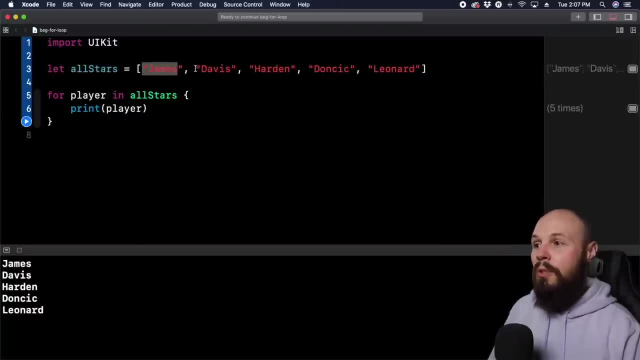 So the first time 줄景 yetmos will go in And I can see discuss this used word: lapashm labour, Am I right? So it makes sense. so the first time through, it prints james. the second time through now player is equal to davis. 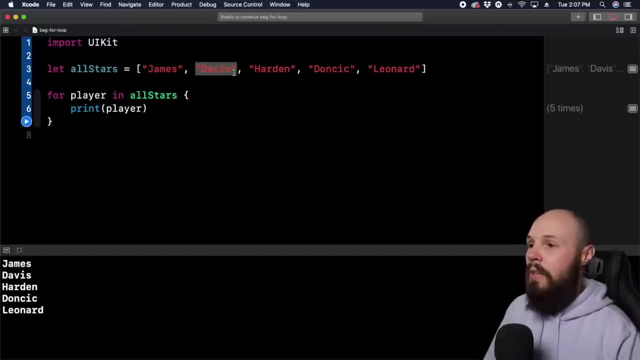 because we're iterating through the array, we're going through each item, um, and the third time, through harden, is the player. so that's how this for loop actually works. and you can even expand on this basic one, like, let's say, we wanted to check, uh, for harden on the specific case, so we 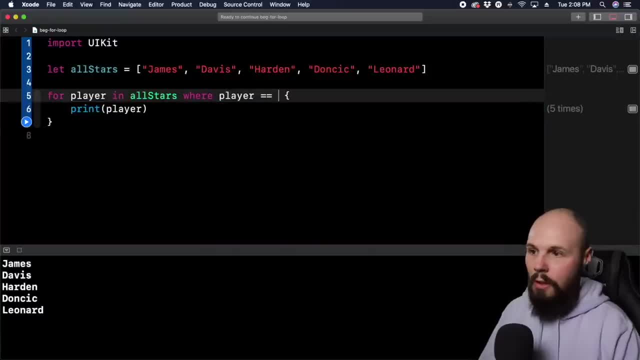 can say where player is equal to harden, right. so again, the way this reads, i know this is kind of a really long line of code for player in all stars. so this means this for loop is going to again go through this entire list, but it's going to check where the player is equal to harden. so the only 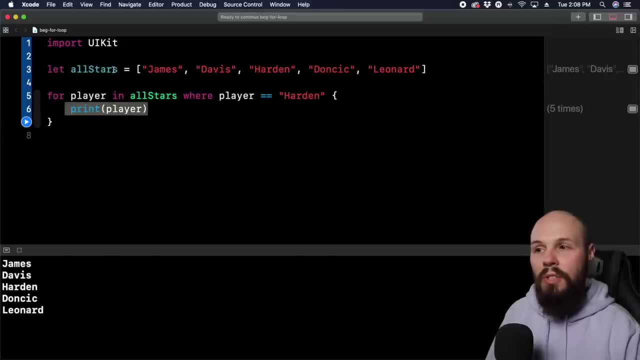 time this code is going to execute is when it's looking through this array. if player is equal to harden, then it is going to print the player. so the only player i should print is harden, because that's the only time it shows up, so let's run it: print harden. so that's a little bit more of an. 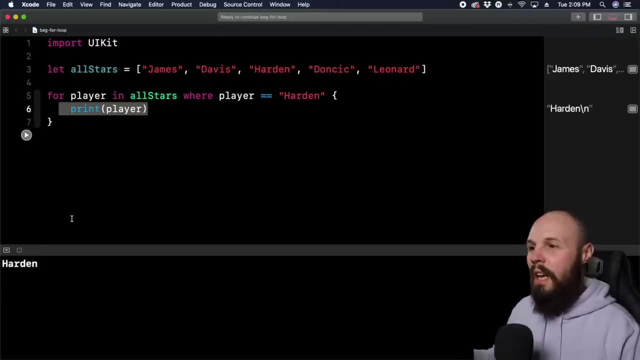 advanced for loop, but it's such an easy example to show and i just like how readable swift's for loops are right for player in all stars where player is equal to harden, like that makes sense, even to non-programmers. i would think so. uh, again that's. 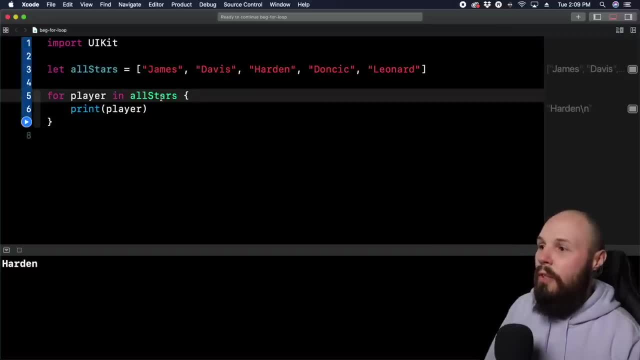 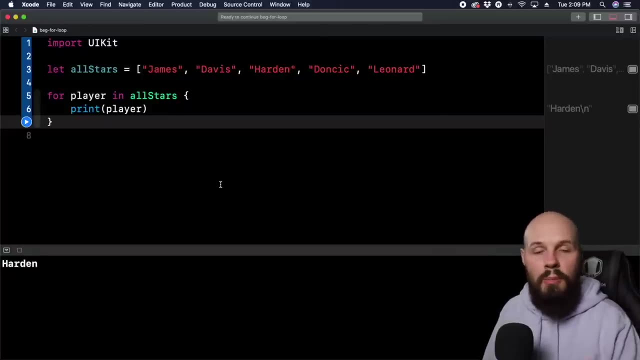 a little bit more of an advanced one. the basic for loop is to just iterate over it. um, like i explained earlier, now that's the first example of iterating over an existing collection- in our case it was an array- and executing some code based on that. the second common example is doing 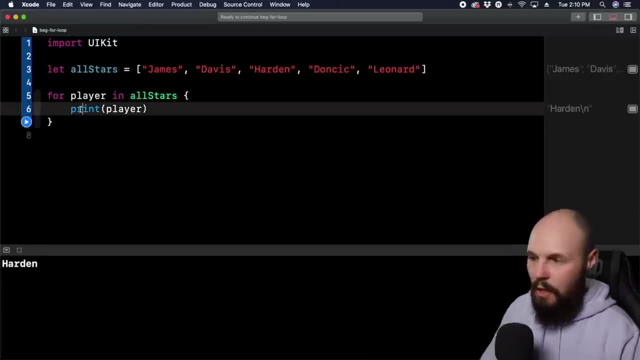 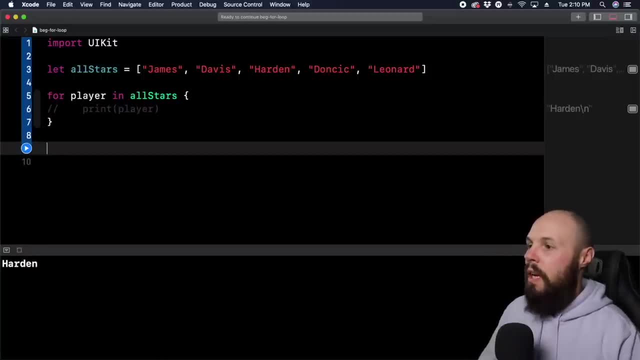 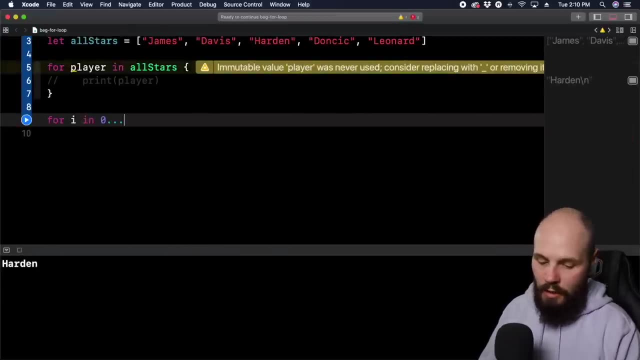 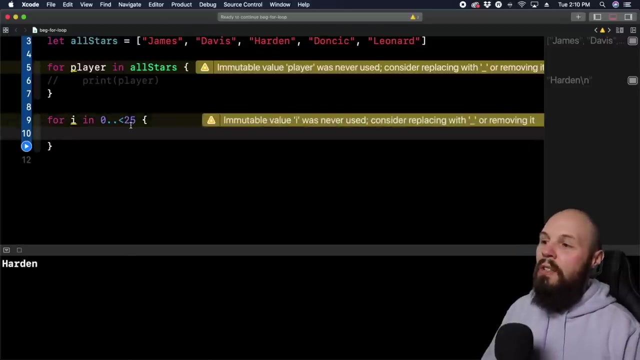 this print statement here, because i don't want to print that out for confusion. so what i can do is i can do for i in and here we can create a range. so zero, dot, dot, dot, uh, i'm sorry, zero less than 25, and let me explain ranges real quick. uh, so that it makes sense. so you can do a range, so i. 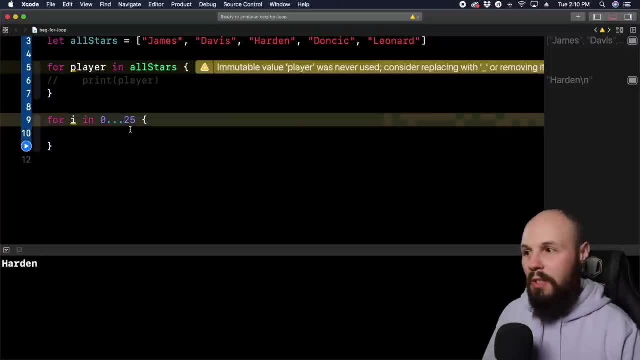 could have done 0 to 25, but that's going to give me 26 numbers because, again, this is how many times it happens. and so if we're starting at zero, that is actually going to run 26 times, because the dot, dot dot will go from start to finish, if you do dot, dot and then the arrow like up until that will. 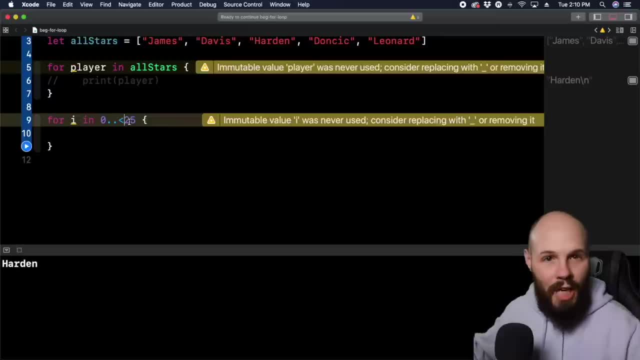 go 0 through 24, which gives me 25 times right, if we're counting zero. um, we're gonna have more on ranges later in the course, but uh, you know sneak peek, it's really tough to like do things in perfect order. um, it's almost impossible right to, like, you know, make sure i didn't show this section. 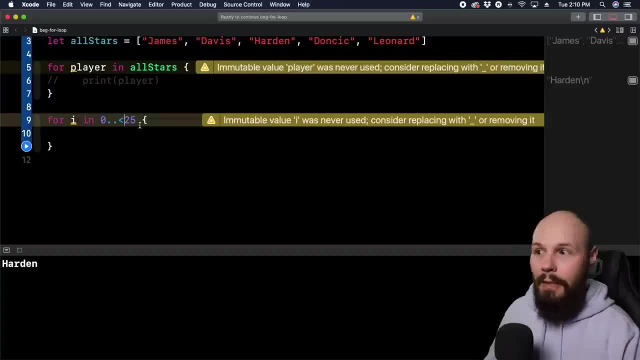 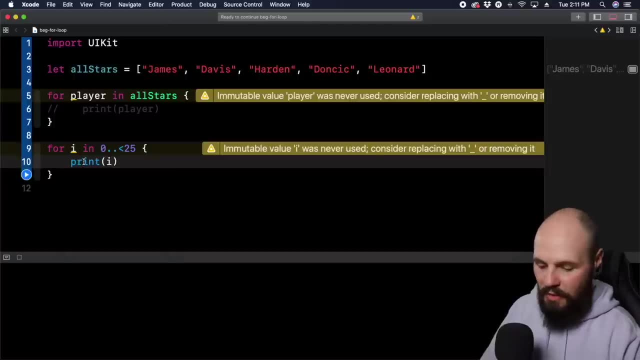 until i showed ranges right, because it's a tangled web anyway. um, so what this is gonna do is, uh, print i and actually, let me, let me go, let me minimize this real quick. you see the error i'm getting from xcode. immutable value of i was never used. consider replacing it with an underscore, remember. 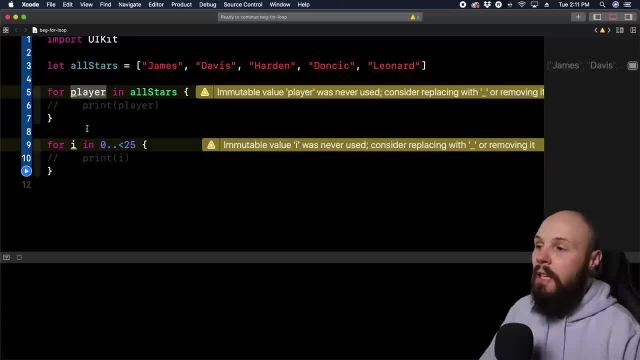 that we're gonna do that in the next example, but, similar to player up here, um, i can name this, i whatever i want. it's just very common in best practice and convention that whenever you're dealing with a count of something- uh, i is pretty much the standard here, but again, you can name that. 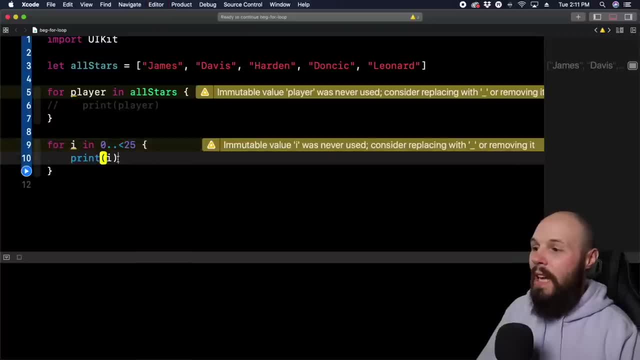 whatever you think makes the most sense. so when i print i, what's going to happen is it's going to print 0 through 24.. because i is going to print 0 through 24.. so when i print i, what's going to in? 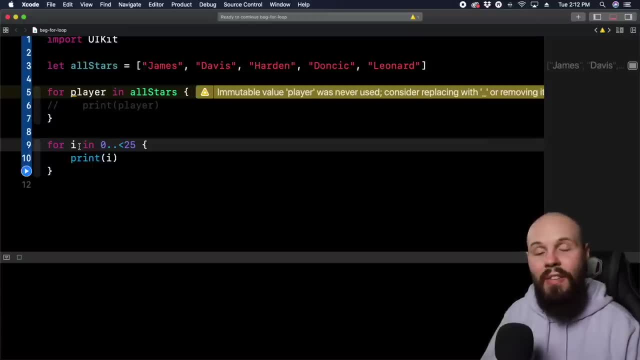 is it's going to print 0 through 24.. because i is going to print zero through 24, because i is going to, i is what i'm printing and i is the counter, essentially, of how many times it's executing. remember this for loop up here in the nba: all stars that executed five times. because all stars. 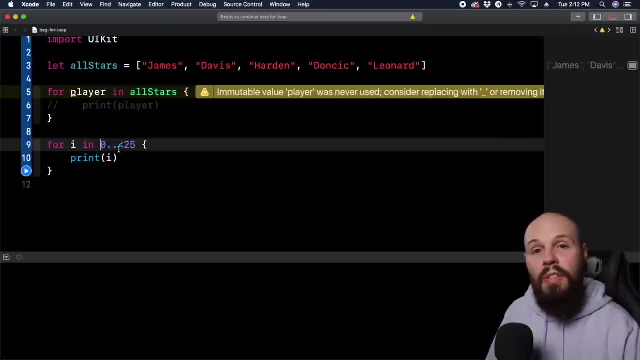 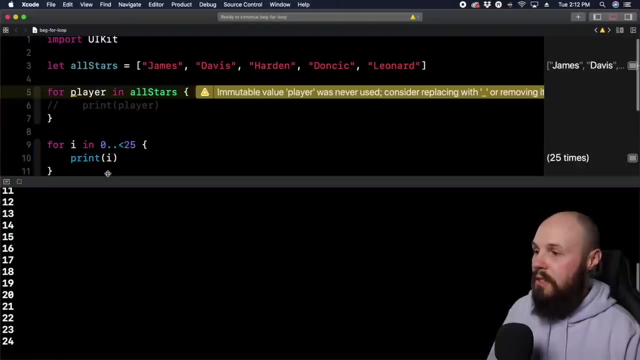 only has five objects in it. well, here i'm saying: run this for loop 25 times. that's what this zero through one less than 25 is. so when i print i it's going to print zero through 24. so that's the 25 items. so let's run it. so there you can see, there's zero through 24. so again the for loop. 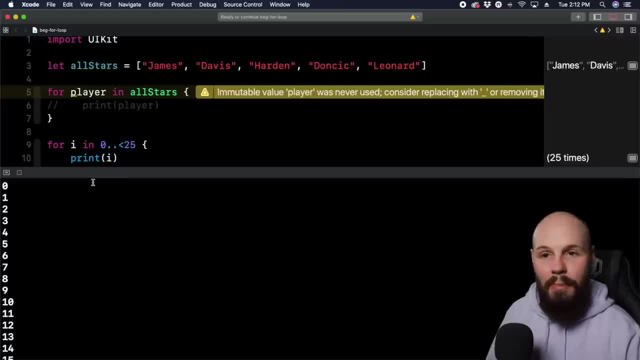 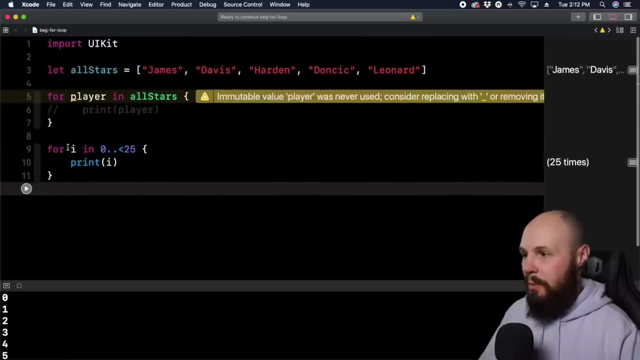 executed 25 times, printing i each time again. that's how many times it's iterating through it. and then over here on the right you can see it went through 25 times. now that's the super basic example. let's actually do something that you might want to do in real life. so let's say we wanted to. 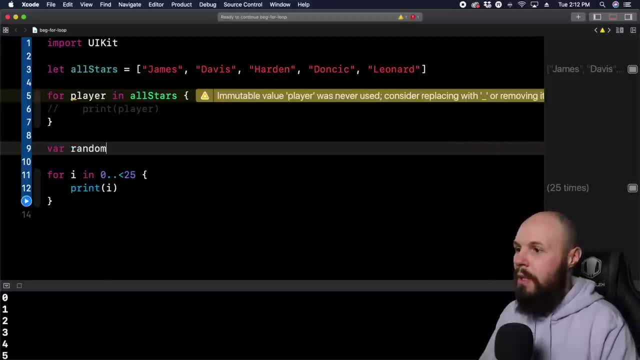 create an array of random numbers, so var at random ints and again we want to declare that as an empty array of int. remember i said you're going to be doing empty arrays a lot like it's pretty common, so this is an example of when we're using that. let me just uncomment this to that: that yellow. 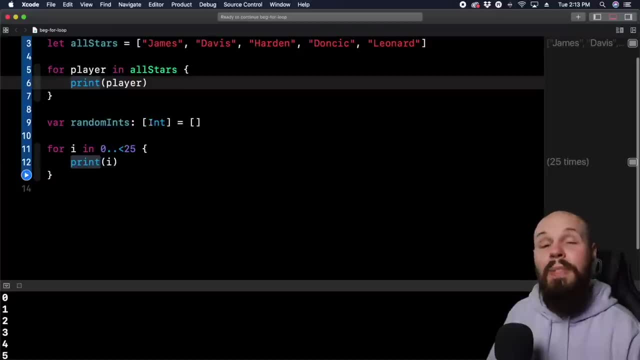 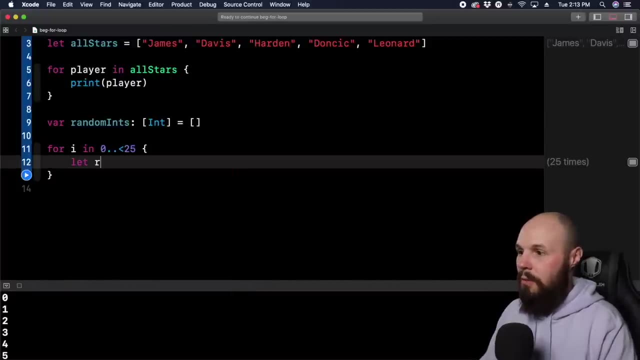 air is annoying me. um, so here we have our array of empty array of random ints. well, here in our for loop, we want to put a random number in there each time. so let's do let random number equals, and this is something we don't actually cover in the course. but uh, int has a random function on it. 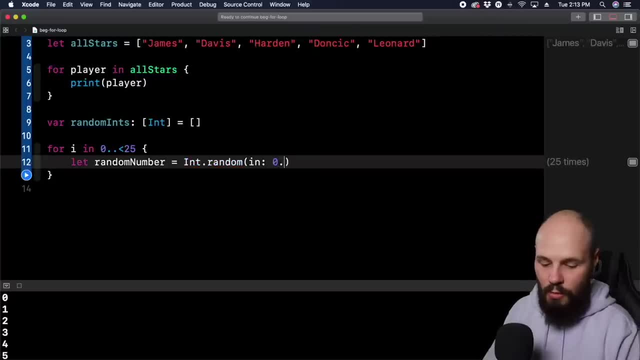 int dot random and we want to pass in the range. we want to do zero one, two, three, one two, three and we want to pass in the range. we want to do zero one, two, three and we want to do 100. so remember that. back to ranges. so i want, uh, any number between zero and 100 to go into my 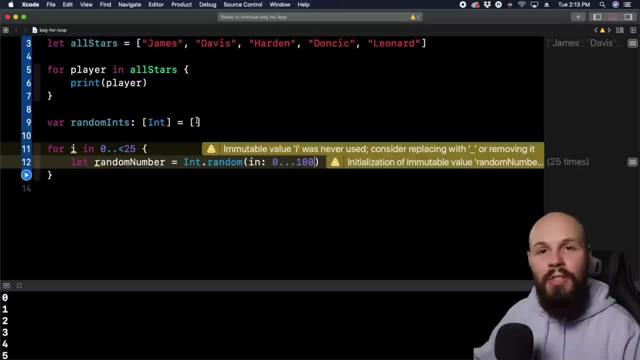 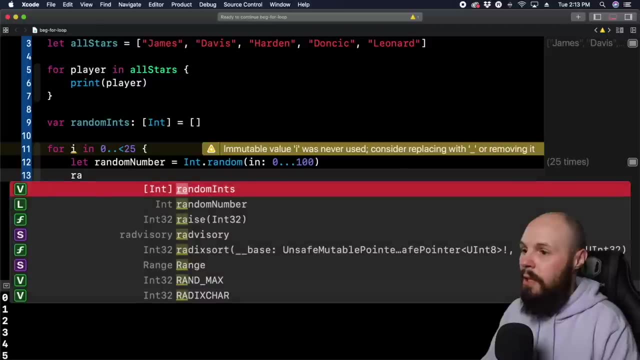 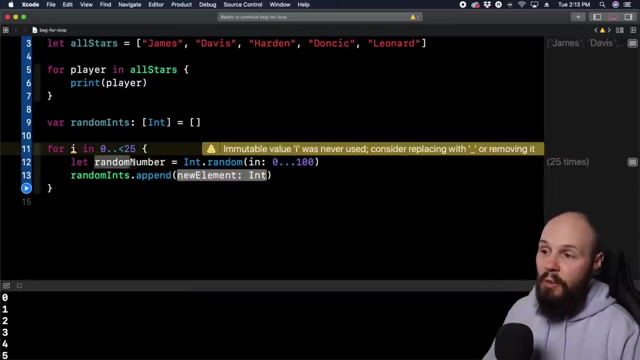 random integers array and it's going to run 25 times. so our random ints array is going to be filled with 25 numbers. so but first we need to append back to our array thing so random ints, which is this array up here on line nine, dot append. the new element i want to append is the: 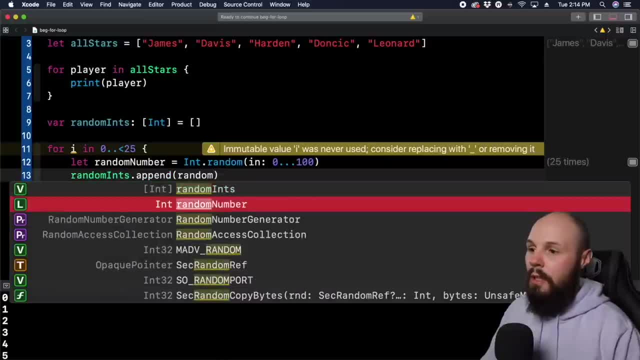 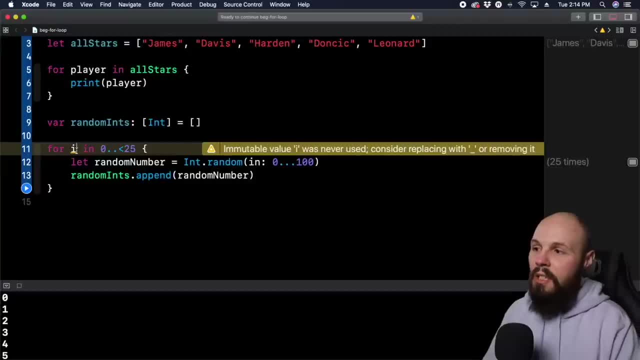 use. this is what i pointed out a few minutes ago. so basically, if you're not using uh, the name variable, it's recommended to just use underscore. so if you see underscore, that means there would have been some variable name there, but we're not using it, so it just avoids confusion. so again this: 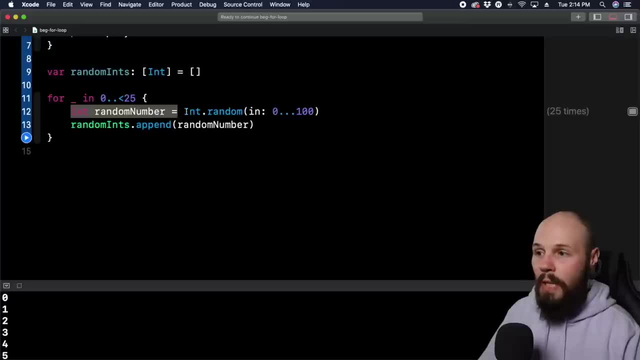 is going to execute 25 times. each time it goes through, i'm creating a random number. that's what. that's what's going on here: zero through 100 and then, now that i have that random number in my variable here or constant, right, it's a let. um, now i take my random ints array and i append this: 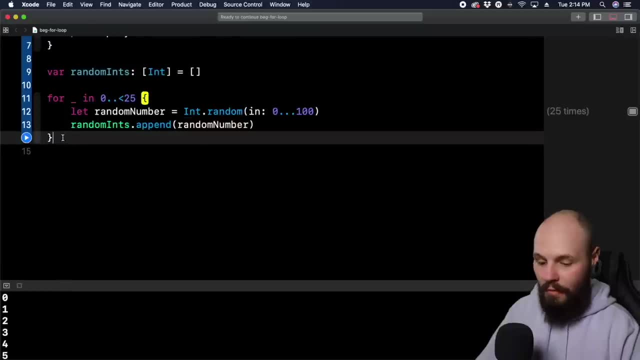 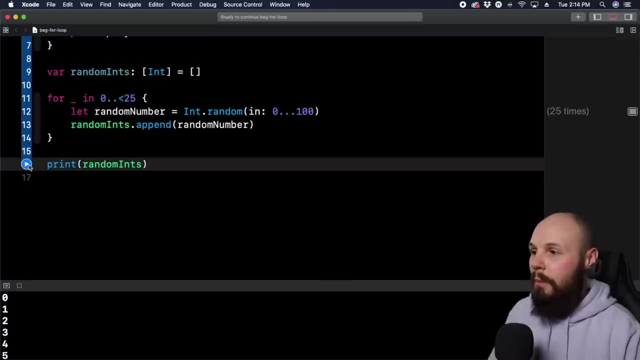 random number and i'm going to do random number and i'm going to do random number and i'm going to that i created right here. so what's going to happen? if i come down here and print random ints, we should see an array of 25 random numbers and again, this is something you may. 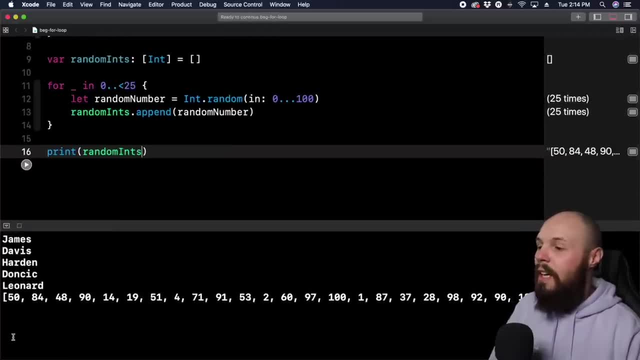 actually want to do for an app. well, after, after it prints off my starting five: uh, you can see 50, 84, 48. right, there's just random numbers, zero through 100 thrown into an array, and we did that real quick using this for loop to create 25 random numbers and then throw them into that array. so 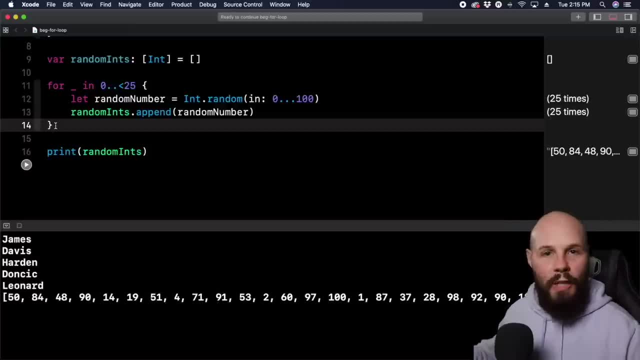 that's the basic for loops. now the topic of loops. uh, there are more like a while loop, a repeat while loop. um, don't worry about those now, because those are, those are more niche. i mean, they're used, but this for loop is used 95 of the time. so this is the. 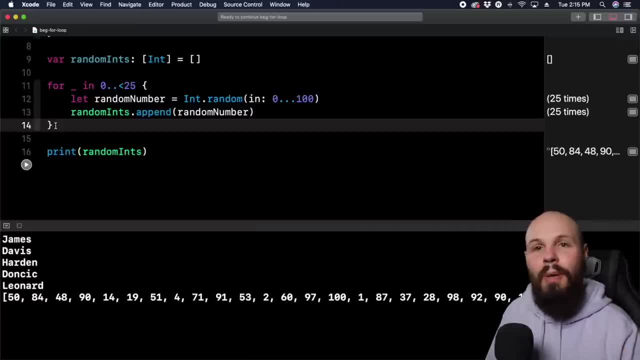 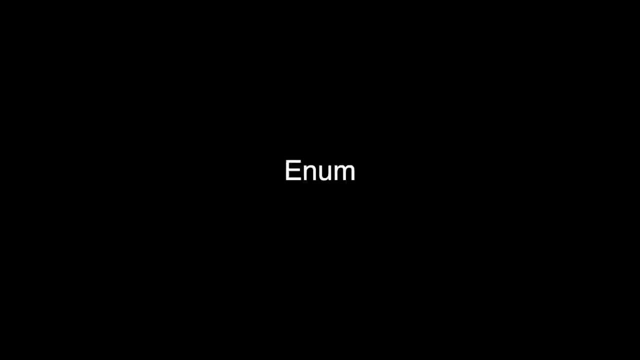 basic fundamentals i want to show, but i will put a link in the description to my video on all the types of loops. if you want further uh information on that, all right, see you in the next video. next up we have enums. some people call it enum it's because it's short for enumeration. 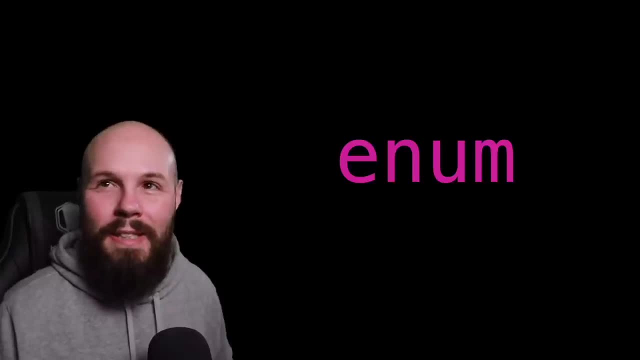 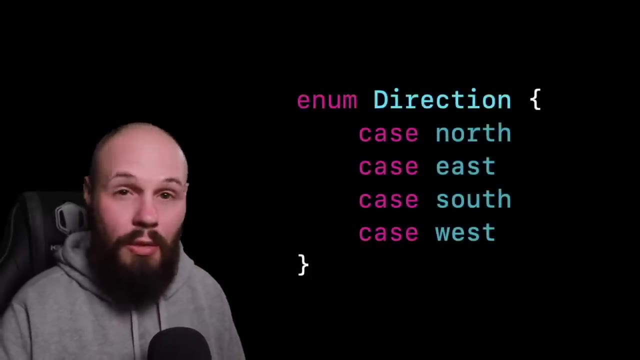 i call it enum, but anyway, an enum is a group of values that are related. uh, here on the screen you can see some common examples. are you know directions- northeast, southwest, right that all makes sense to be grouped together. sometimes you have you know days of the week: monday, tuesday, wednesday, etc. 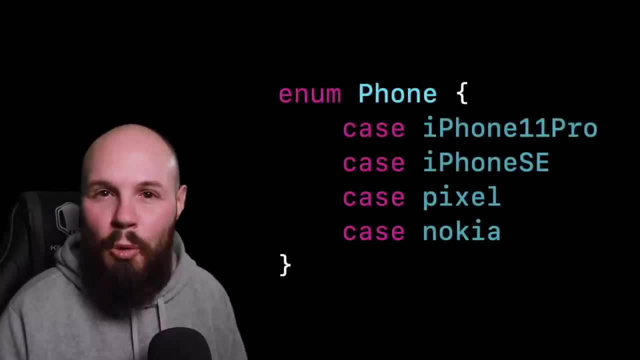 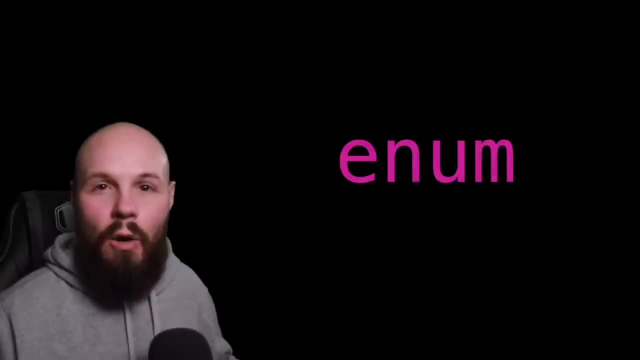 right, that makes sense to be grouped together. uh, we're going to use an example based on phones, right, iphone, you know, google, pixel, uh, etc. so the basics of an enum again are a group of values that are related that you put together in an enum and in this. 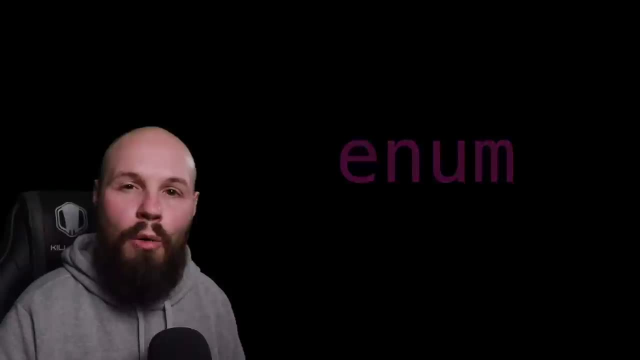 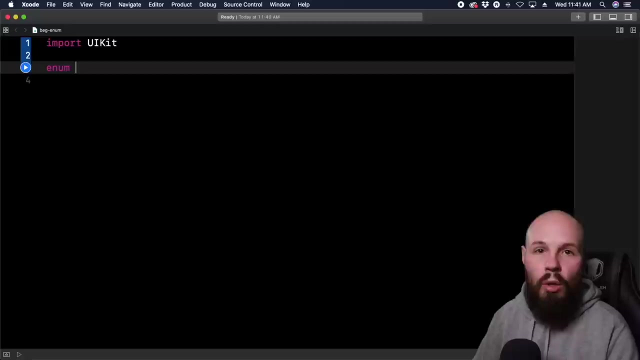 video, i'm going to show you some examples of how to use them, uh, so you can see how powerful they are. so here in the brand new playground again, go ahead and create that on your own. uh, to create an enum, you just do enum and then you call it something. so we're going to call this phone. 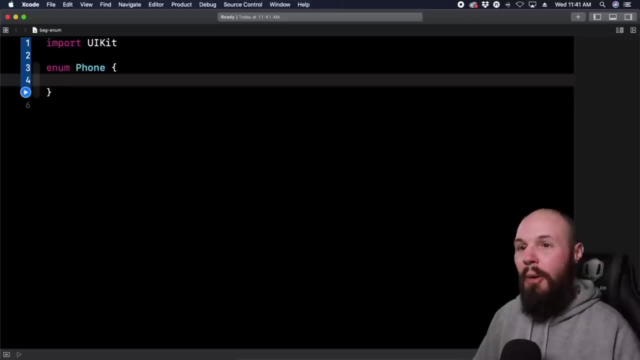 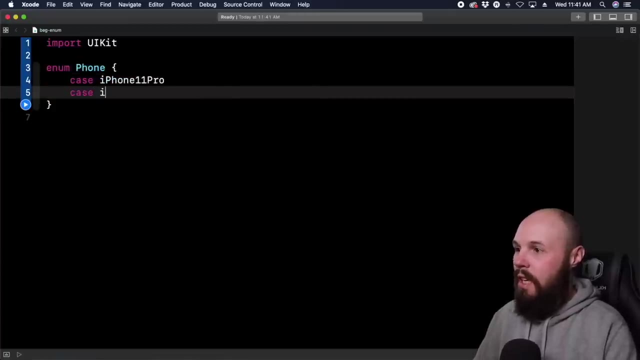 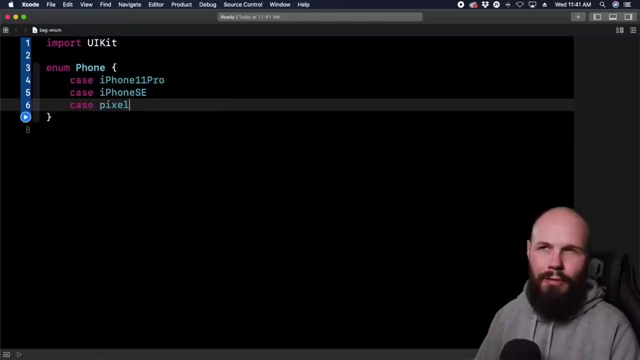 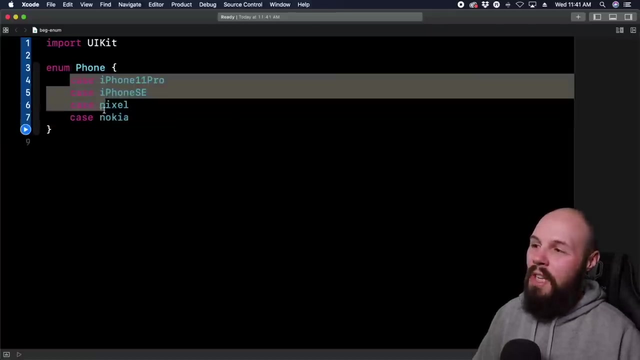 and then open bracket, close bracket to you know, create the scope. now, each enum has a case, so you do: case iphone 11 pro case, iphone se case, uh, you know, pixel, i don't even know what number, the four, we don't mess with that, right, uh. and then case, uh, nokia. now, uh, i listed all these out with. 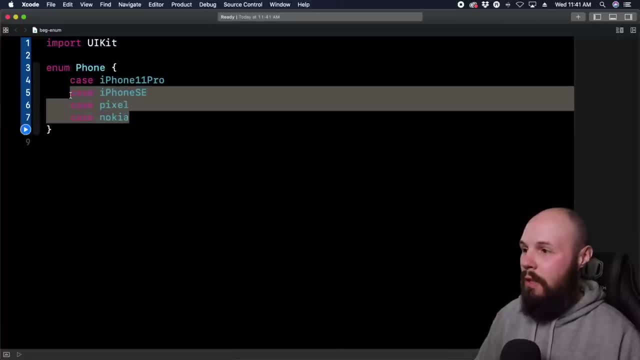 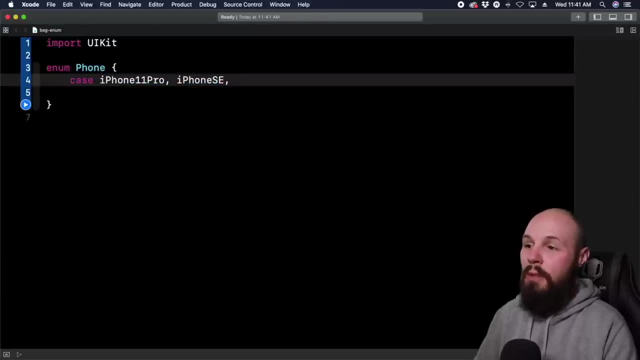 you know which each line uh has a case. you can. however, i'm gonna cut this so i can paste it back. you can do iphone uh, iphone se. you can do comma separated uh, to put it all on one line, if you like. i'm not going to type out the rest of the phones, but i could have listed those out all on one line. 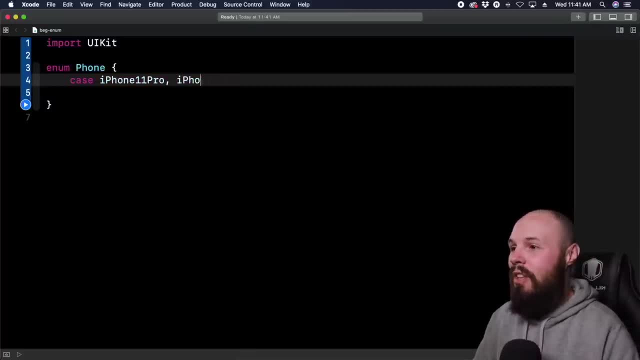 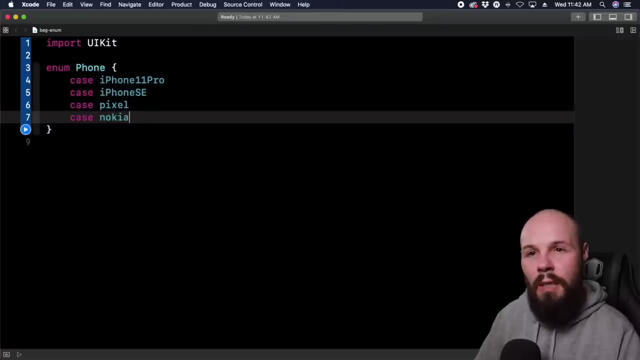 so if you see an enum declared like that, it's the same exact thing as having them all out on one line like this. now i'm going to leave it like this because, as somebody just learning enums, i think it's better to visualize it as like separate cases when they're all on separate lines. so now i'm going. 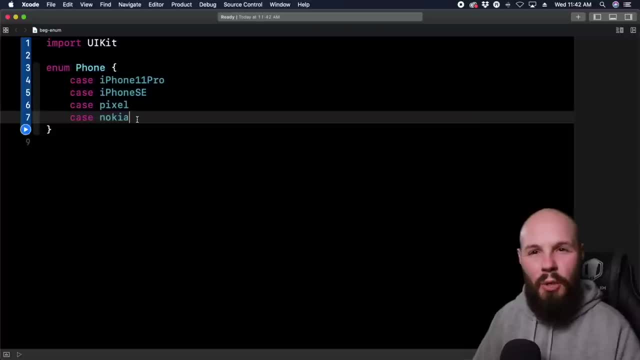 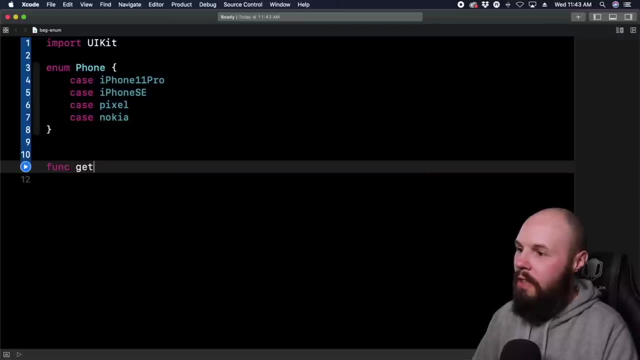 to show you two examples of using enums and you can see how they can make your code a lot more readable and clean. and to do that we're going to create a function, so that function is going to be funk. get sean's opinion and then on and remember: this is the argument label and then our parameter. 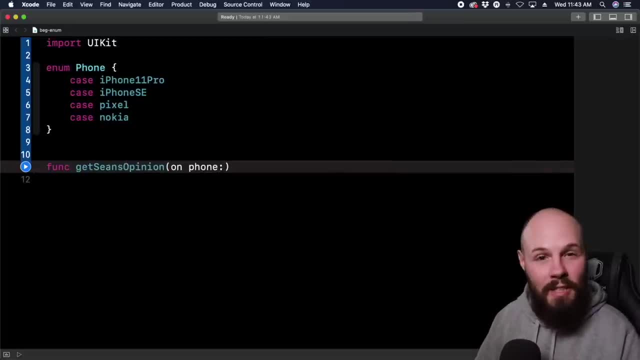 label: it's going to be phone and then the type this takes in. remember we talked about you know, it could be an int or a string. well, now we have our own custom one called a phone, up here on line three. so this is going to take in a phone, that's. 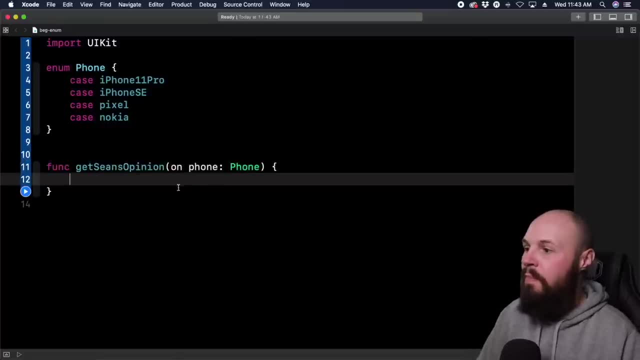 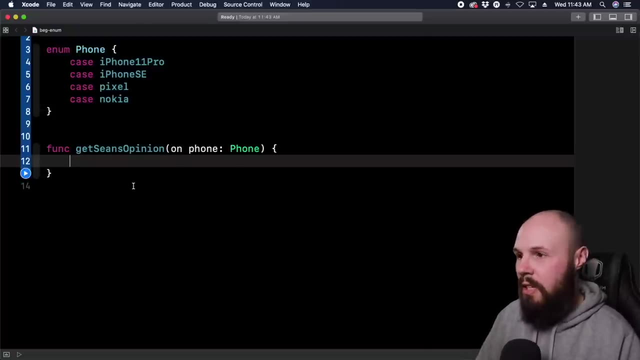 what we're going to pass in again, open and close parentheses to declare the scope of our function. so again, our function is get sean's opinion on phone and we're going to pass in one of these phones. you're going to see how we use this in a second. actually, you know what? let's go ahead and. 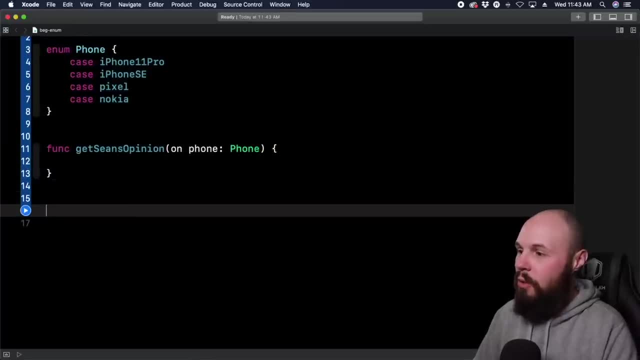 write it right now. um, so, in order to use this, i can do get sean's opinion on phone again back to how readable swift can be, and the phone i pass in is one of these cases, and you can see i can do dot and then i can get the options in my enum. right, you can either be. 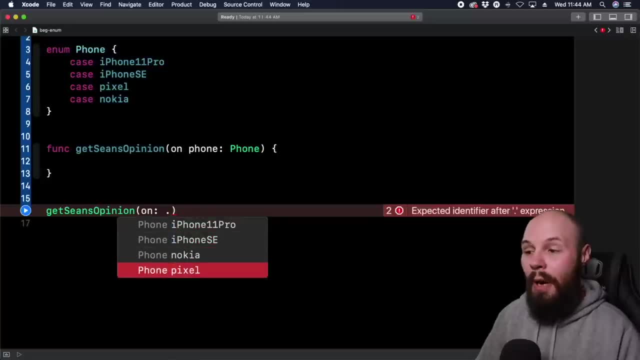 an iphone 11 pro, iphone se, nokia pixel, etc. but i only get these four options because, again, i've declared this enum with only four cases and that's why enums are a group of you know related values. again back to the other examples. you know northeast, west, south for directions, uh, or days. 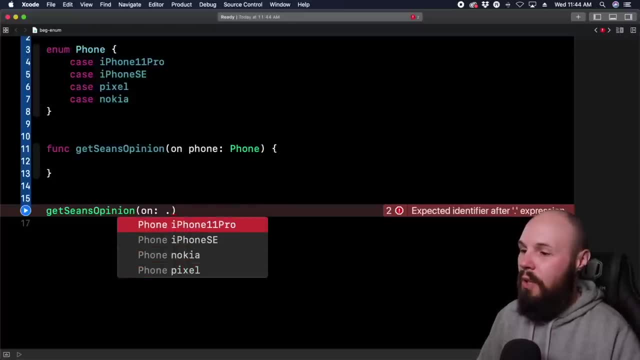 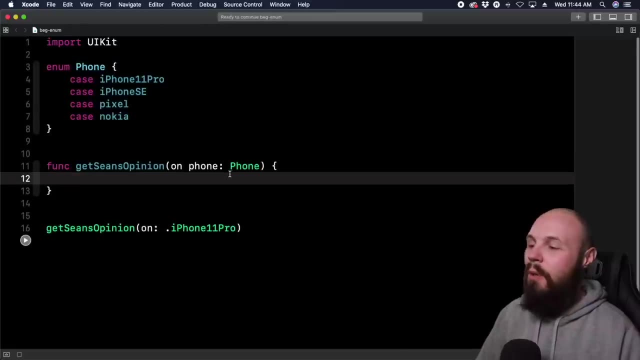 of the week, uh, etc. so we want to pass in the iphone 11 pro and we're going to pass in the iphone 11 pro. now, if i run this, nothing's going to happen, right? because we haven't written any code in our function right here. so let's go ahead and do that. and i know i keep going back to this. 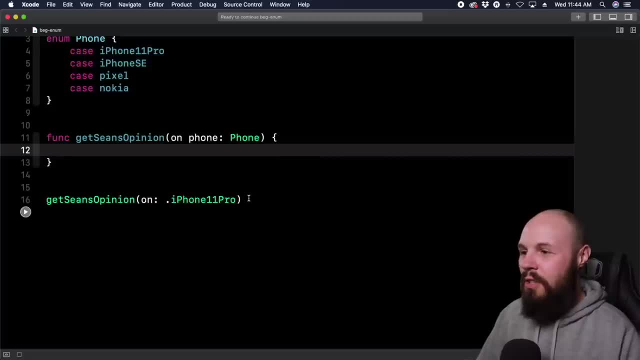 but i just love how you can make swift so readable, like right, get sean's opinion on iphone 11 pro. i mean, that's like a human readable sentence, right? it's not even like code. uh, anyway, i digress back to writing the logic in this function. so we're going to build upon a previous video where we did. 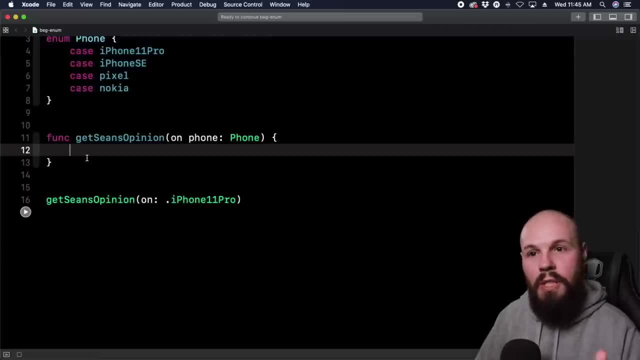 if statements right because there's multiple paths. right, we talked about how you can do the if else and then else if to go down the line, and then we're going to pass in the iphone 11 pro multiple paths. but we have four paths to take care of: iphone 11 pro, iphone se, nokia and pixel. 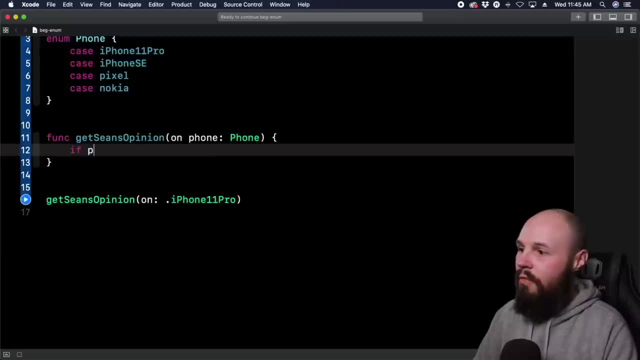 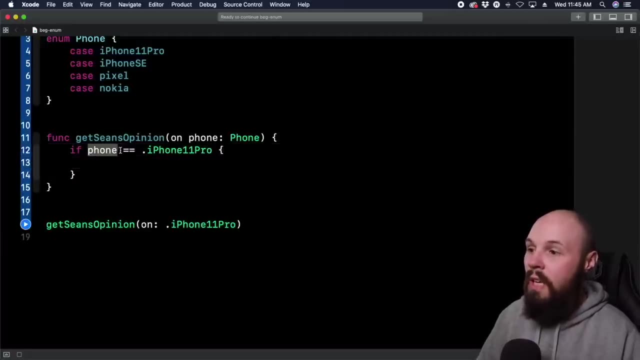 to get sean's opinion on each one. so let's do that. so if phone uh equals equals, dot iphone 11 pro, we want to do this, and now again, real quick. this phone is what i named, my parameter, so phone here. so now i have access to this phone within the scope of my function. right? so that's how we're. 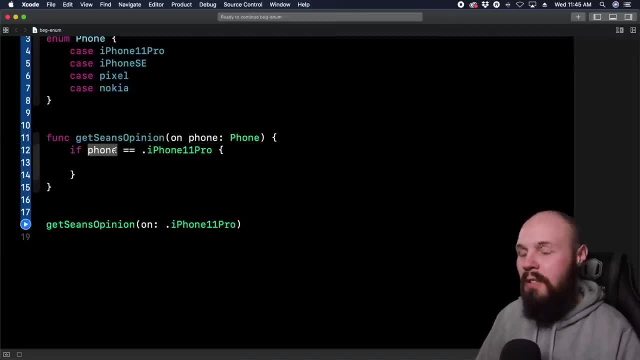 accessing it here and i like to go back and reinforce and repeat stuff from previous videos just to really drive the point home because, like i said, i know in the original videos for some of these i went over them very quickly, but that's because we're going. 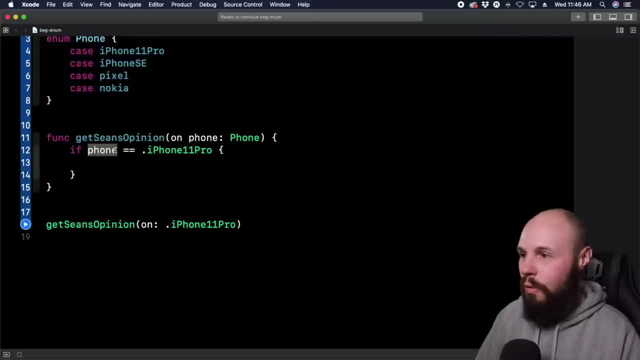 to use them throughout the course. and again, you're going to get plenty of chances to really utilize uh these skills. so if phone is equal, to remember the double equal sign, iphone 11 pro- we want to print uh, this will be my next phone. it won't be because i'll wait for the iphone 12, but whatever. 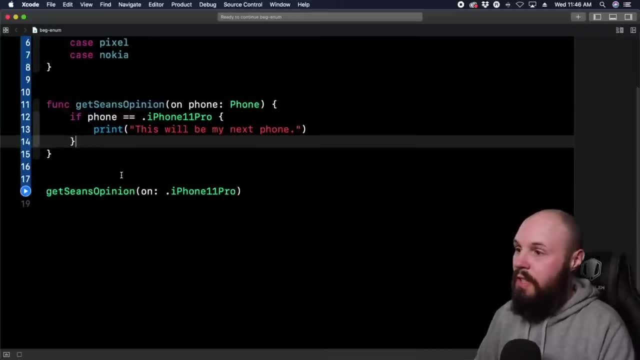 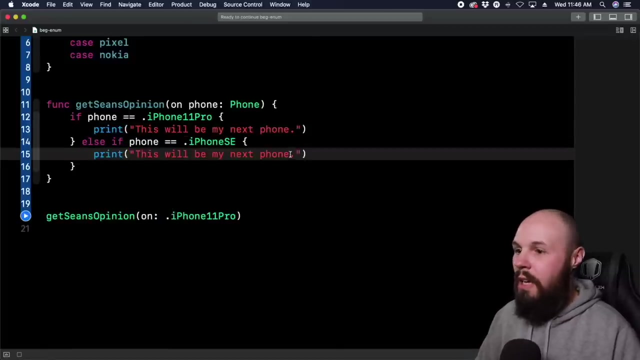 and then now multiple paths with the if statement. this is review from a previous video, so else, if uh phone equals equals dot iphone se. we want to print out something else and i'm just going to copy and paste this, this print statement, because i don't have to type it every time: uh, and now we will say: uh, i dislike. 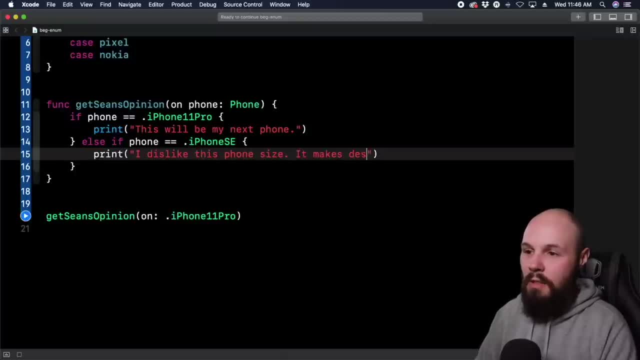 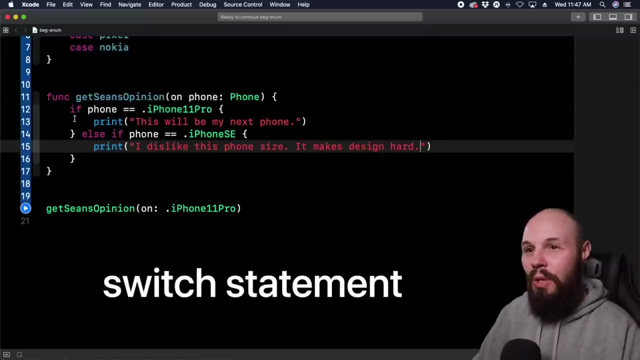 this phone size. it makes design, design hard. that little small phone size, uh. but so some of you who have maybe seen swift before, maybe saying like this should be a switch statement. you are correct, but i don't want to get ahead of myself and i want to reinforce the switch statement and i want to 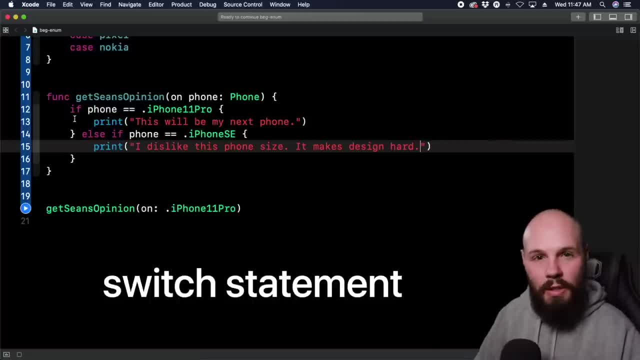 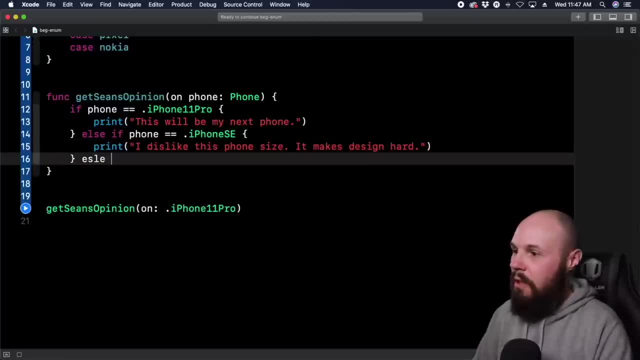 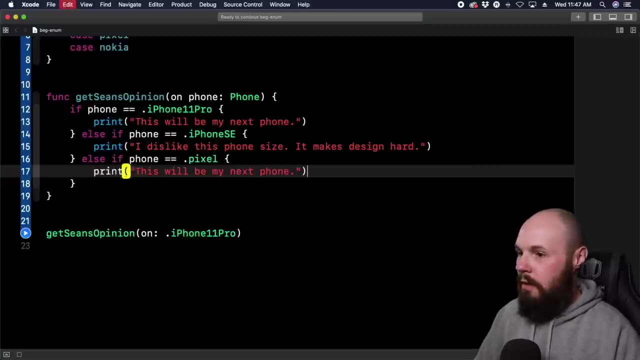 uh, if else, if, get practice at that. in the next video we're going to talk about switch statements and how you can clean this up more on that in a bit, all right, so the next path we want to handle is else, else. if phone equals, equals, uh, dot pixel, and i'm going to say, uh, hardware is great, android. 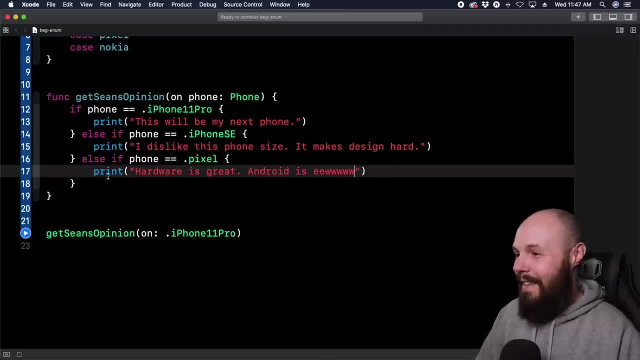 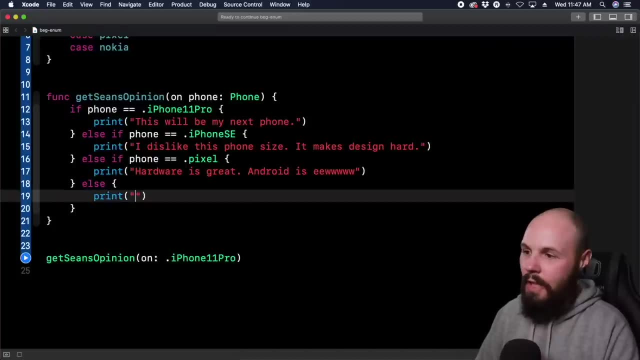 is: ew, don't like android. uh, and then else again uh can be the catch-all and put the print statement in there and uh, this is like that old nokia phone. right is can't be broken. classic, that old nokia phone. so again, how this function reads is it's going to get sean's opinion. 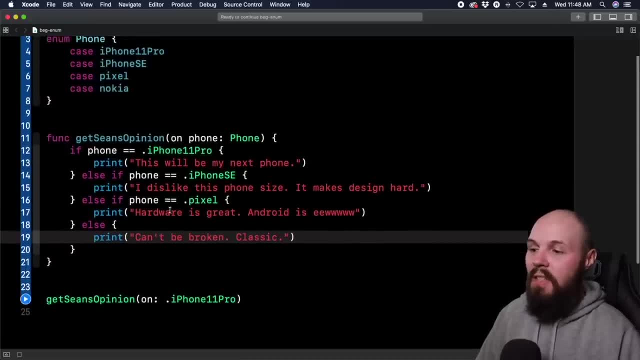 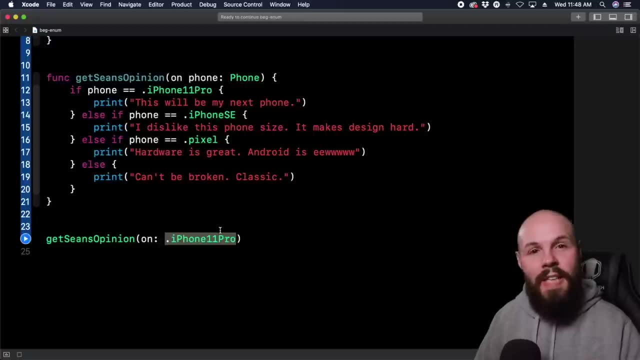 we're going to pass in a phone using the enum right and the enum makes it nice and clean, so i can just do dot iphone 11 pro. remember before we were passing in strings and we had to type in the string. the danger with a string is that if you make one small typo, uh, your code's going to. 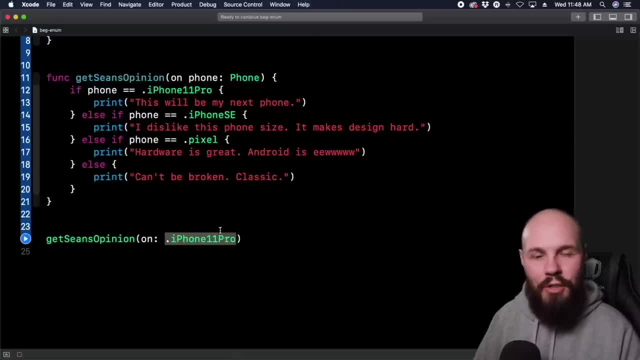 break right, and so if you're typing strings all over the place, that's very fragile. um, we call it stringly typed. that's not an official swift term, that's kind of just a some slang. but you want to avoid stringly type stuff because again, one small typo everything. 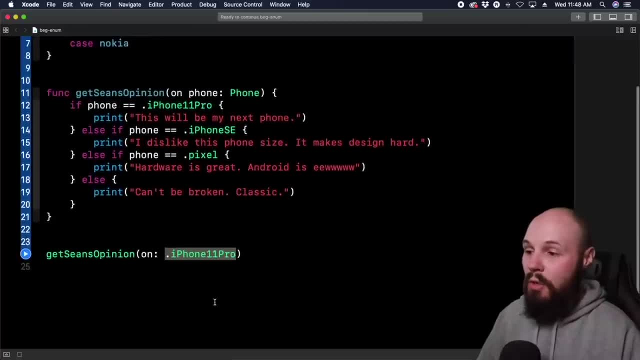 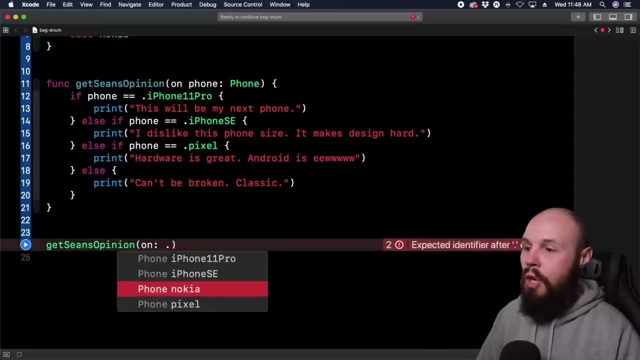 breaks. so putting things like this in enum uh will make it. so you get the autocomplete uh, like you saw here, to where i can just type in, you know, all right, i get the autocomplete here. so we're going to. we're going to try the nokia first, so let's run this and we're passing in nokia here. 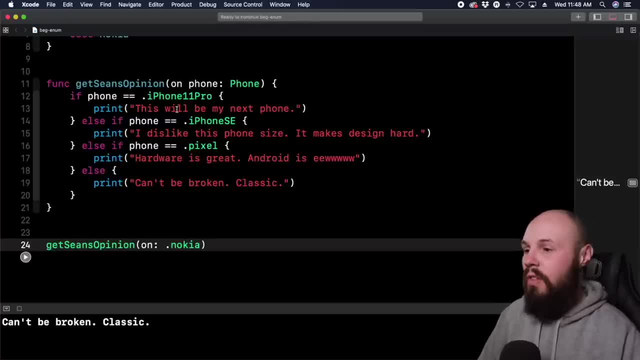 on the phone thing and then, you see, it goes through our if statement, like we did in the previous video, and it determines that i'm on the nokia phone. so it prints out: can't be broken, classic. and let's just test one more. let's pass in the iphone se, run it again, and you see, i just 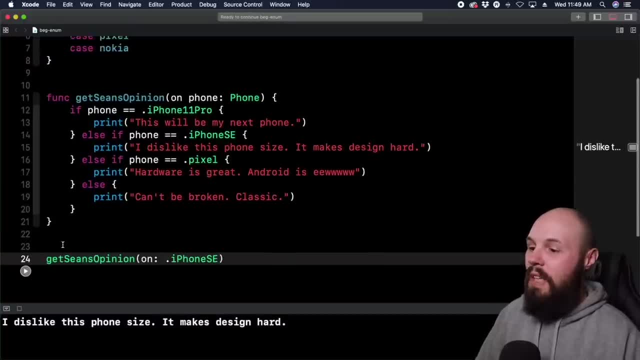 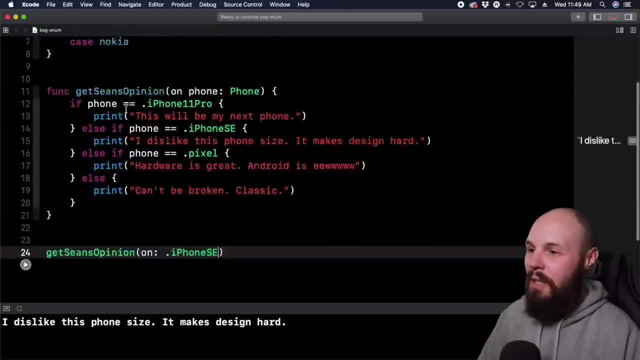 like this phone size. it makes design hard. so you can see again, the power of enums really cleans up your, your code, makes it nice and readable and it's also easy to understand. right, you have your list of phones, uh, up here now. if you look at this function, uh, it's kind of kind of sloppy kind. 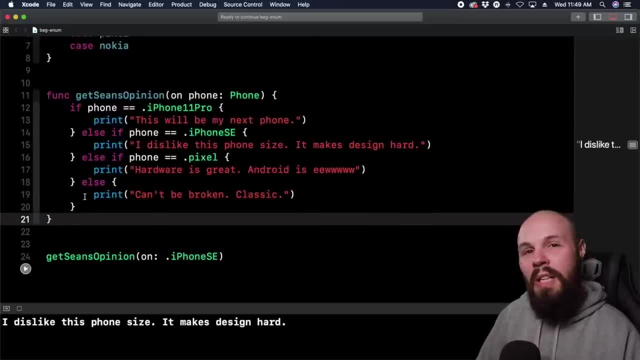 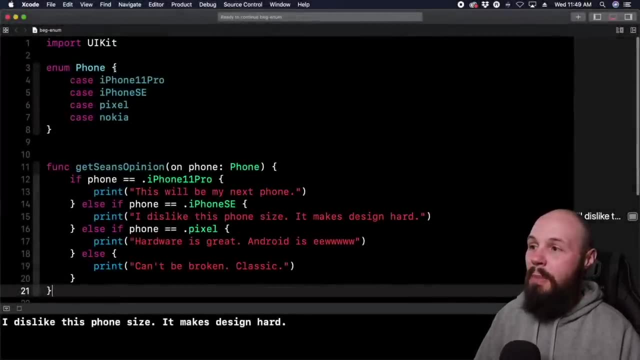 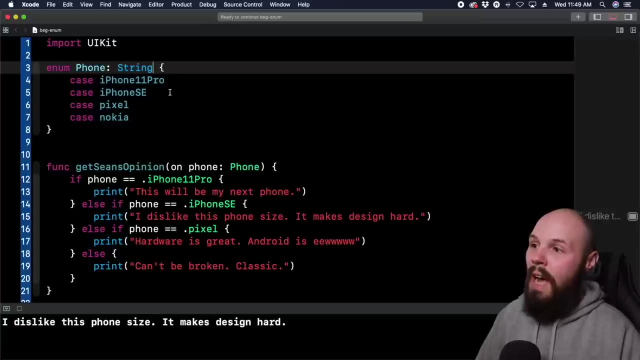 of messy. like i said, we can fix it with a switch statement. but we can actually make it even cleaner by using raw values on our enum. so up here in our enum we can actually give it a type. so right now it's just generic, right, a phone? we can say a phone has a string raw value. so now 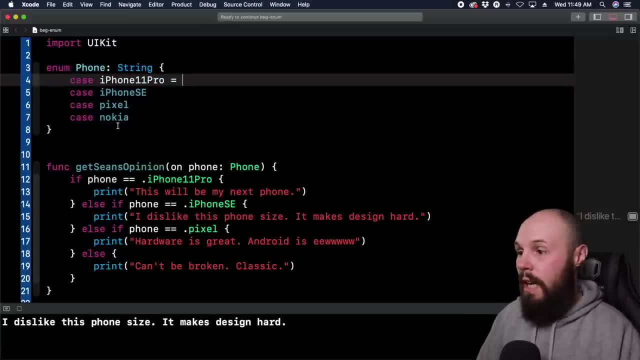 i can say: the case for the iphone 11 pro is going to equal and it's because we declared it a string. i can take this string and put it up here. so now the case of iphone 11 pro has a raw value attached to it and that raw value is a string and that string is: this will be my 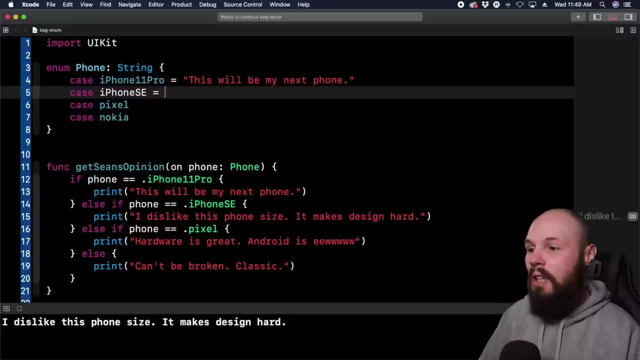 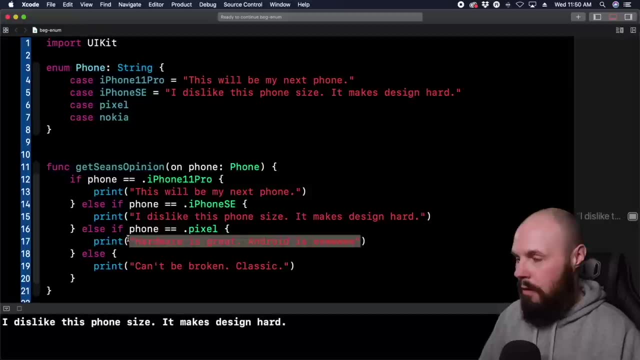 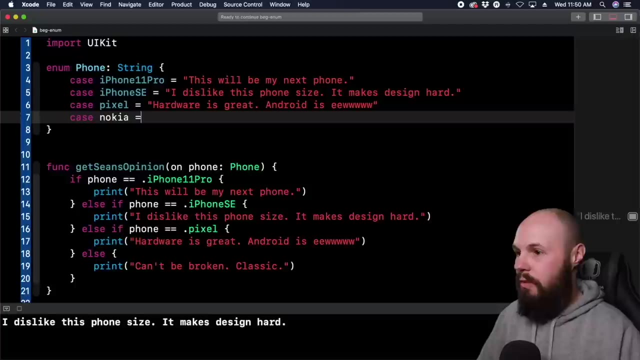 next phone. so let's go ahead and do that for the rest of them and you'll see how it's going to clean up our function. uh, very nice here. so do this: maybe copy equals. maybe copy equals, command v. okay, cool, so all of our strings are up there as uh, and if you don't know me you'll know i like to do this. 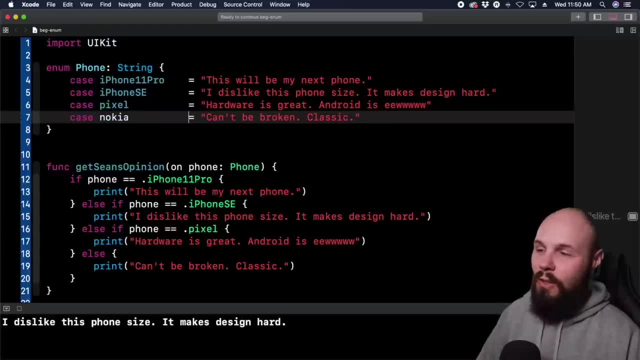 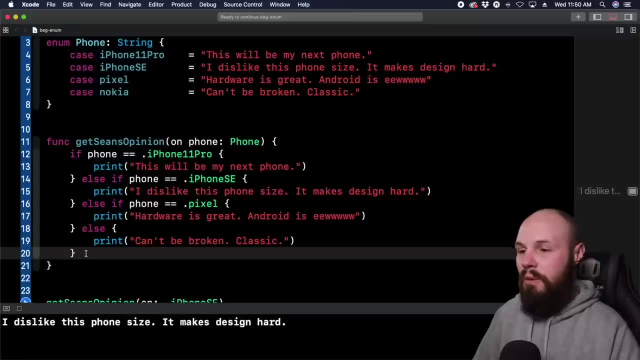 i like to line up my equal signs to make my code uh, look neat. you don't have to do that, that's a stylistic choice. but now this, this kind of if else statement- and i'm teaching you this as a beginner, because it is foundational knowledge- but the honest truth. 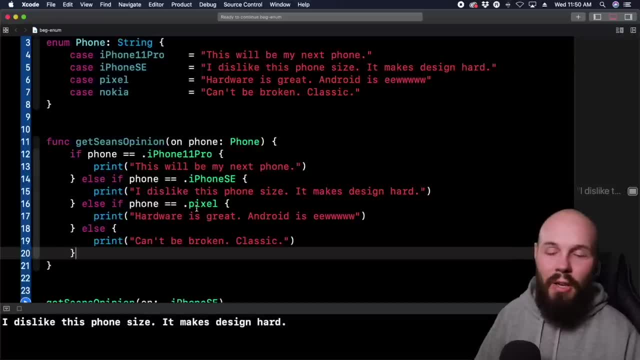 is if you find yourself with a very long if statement, if else 99 of the time, there's going to be a better way to write that, and that's kind of what i'm illustrating right here. so usually, if you see this, this is kind of sloppy code. it's usually the sign of a beginner. 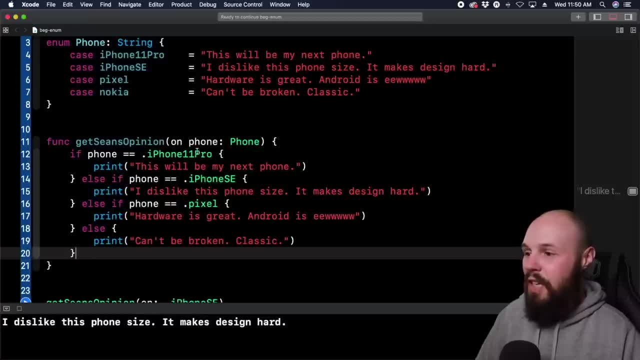 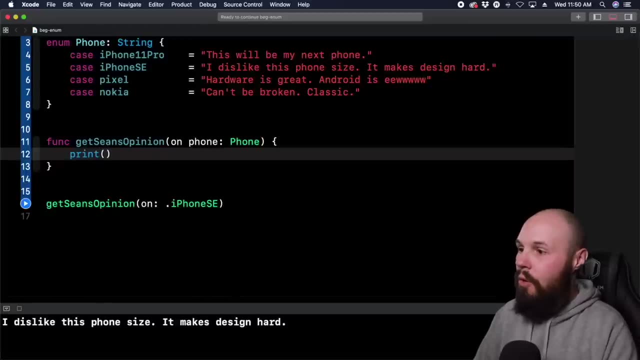 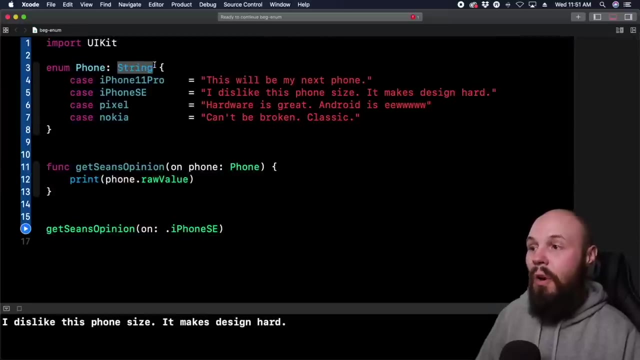 so we're going to clean this up. so, instead of having the if statement and checking, we know we have a phone, right, so i can just do print and then, uh, phone dot raw value. enums have a raw value, right, so this right here. remember we said this phone has a raw 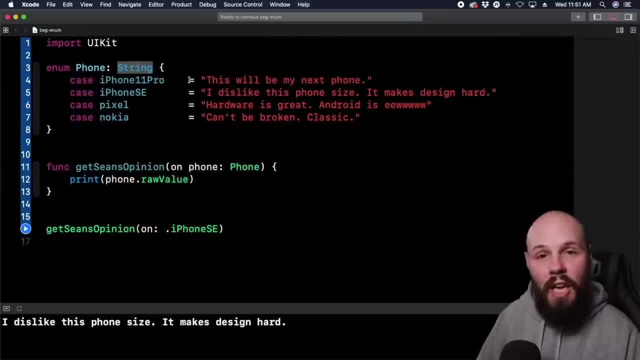 value, that is a string, and then on each of the cases i gave each case a string for a raw value. so now, instead of having that crazy if statement down here, we can just print phone dot raw value and it's going to print the string. so to prove that let's not do the iphone se, let's do the pixel. 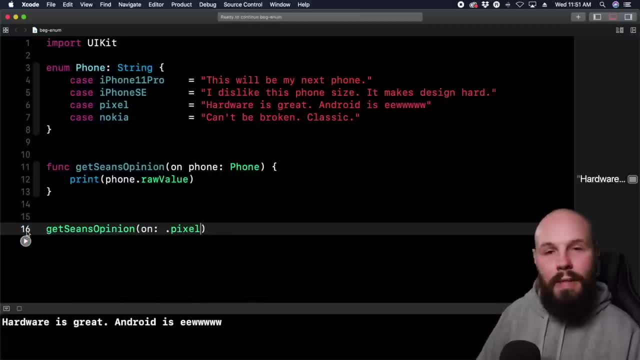 and run it. hardware is great, android is used. so you can see, because pixel was passed in, this is pixelraw value, and pixelraw value is hardware is great, android is ew. so that's basic enums. uh, enums are actually a pretty deep topic. there's a lot more you can do with enums. associated values: 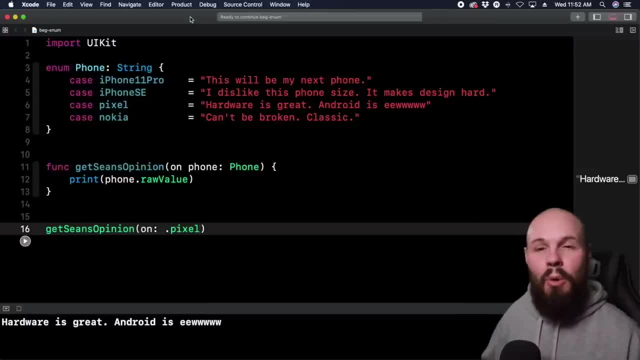 uh, enums can have functions attached to them. again, beginner course, this is how you're going to use enums, uh, the vast majority of the time. so, uh, just start here with enums. again we have the different cases. uh, you can pass. in the case of the function, it makes the code nice and clean and very readable. 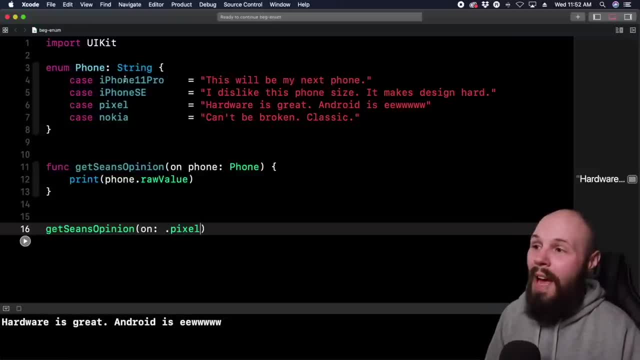 and then also we can assign raw values to them. so again, when we pass in the case iphone 11 pro, it has that string attached to it and then we can access that string by saying phoneraw value, as you saw in this latest example. all right, that. 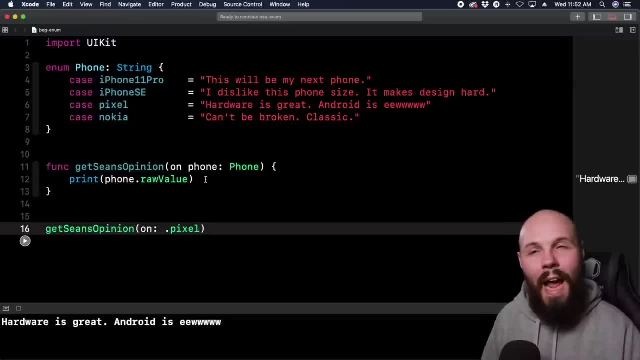 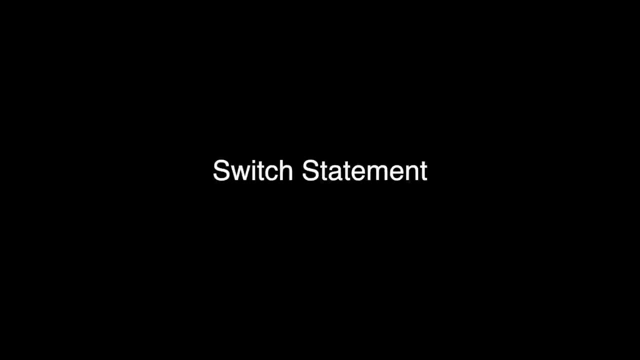 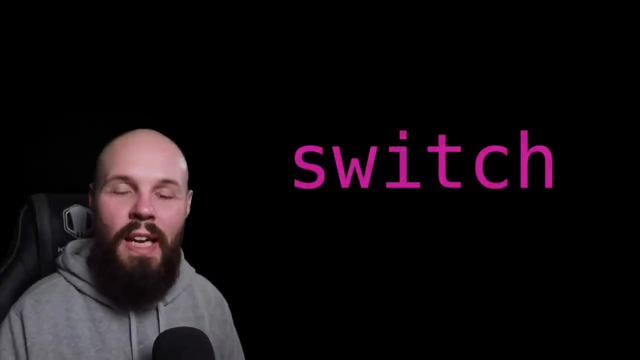 wraps up enums. we're going to move on to switch statements, which don't have to be paired with enums, but oftentimes they are. so let's move on to that video. in the last video we had that sloppy big if else statement. uh, in this video we're going to talk about switch statements and how we can. 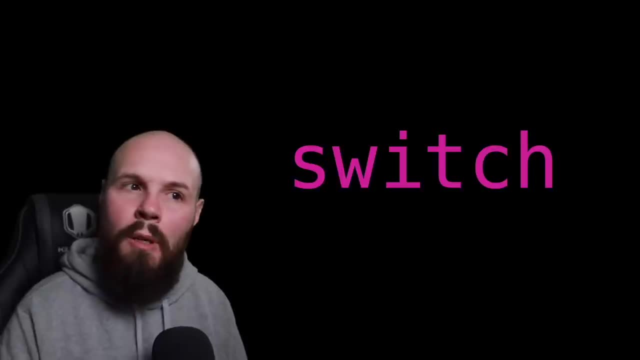 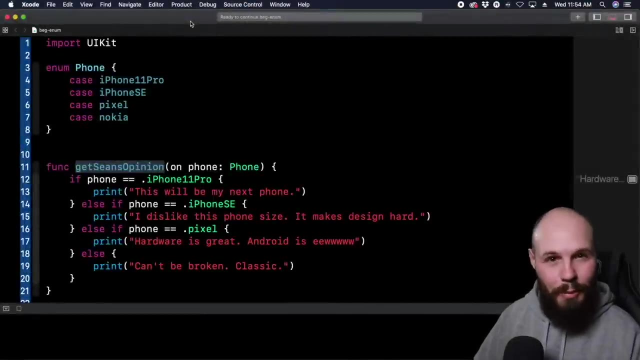 do that. so, like i mentioned last time, switch statements are often paired with an enum, but they don't always have to be. let's dive into an example to show you how to use this. so here we are in our previous playground. hopefully this looks familiar. it's from the last video where 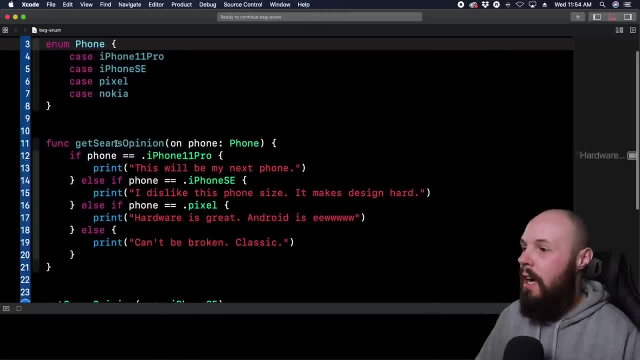 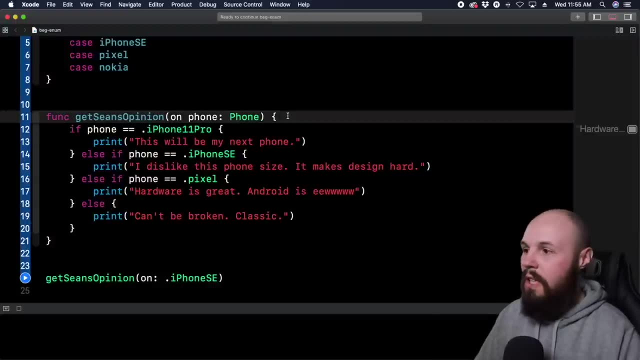 we have our enum of a phone. i took away the raw values because we're going to showcase the switch statement. um, what we're going to do here is replace this if uh else stuff with a switch statement. so what i'm going to do, so i can copy and paste to save all the typing time, is make some. 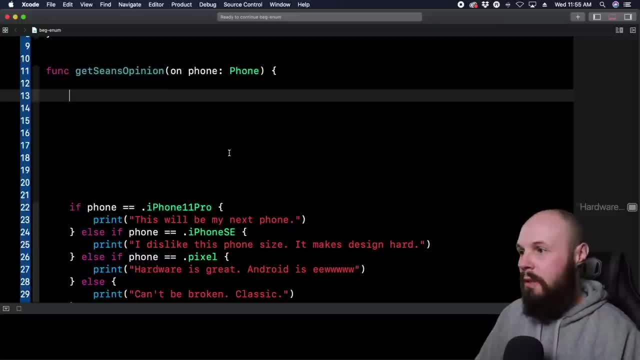 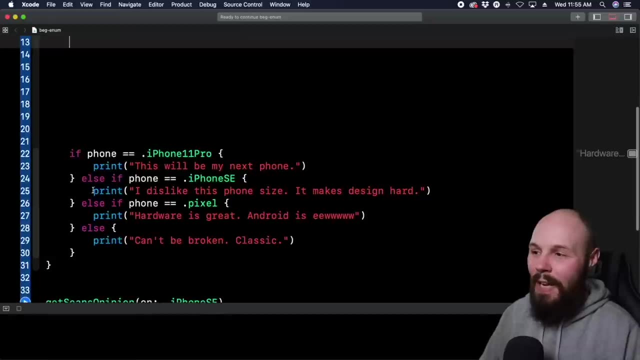 space down here and we're going to create our switch here. i'm going to go ahead and type in the end of deleting that bottom part later, but i just wanted to make space so you can see it. uh, so to create a switch statement, and again it's. it's basically just a cleaner way to write this. 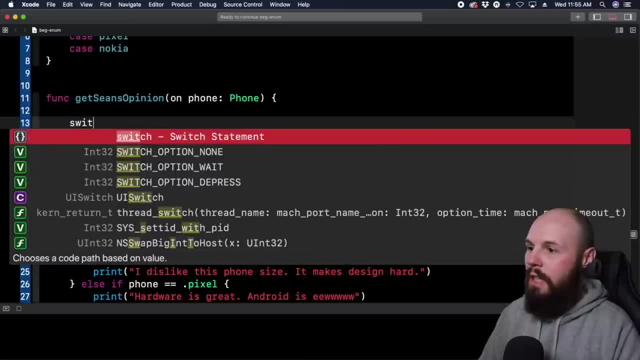 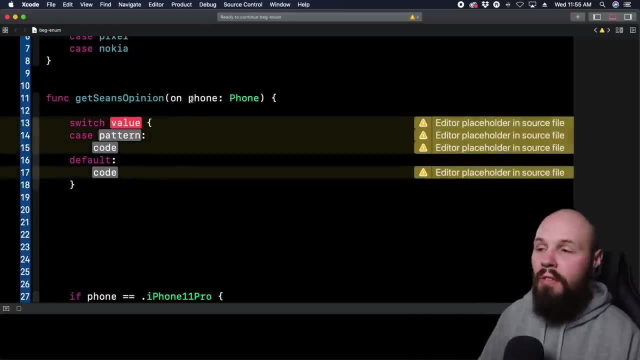 and it's more readable. so let's do that. so switch, and then i'll hit enter to get the basic switch statement. um, we'll kind of go through this. so the value here is we want to switch off of our phone, we want to handle all the cases of a phone, so our value is the phone. that's what we're going to. 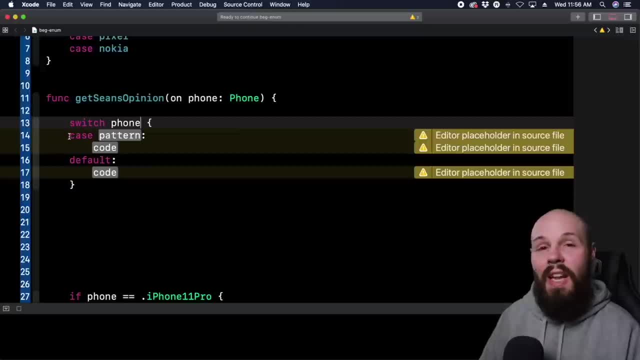 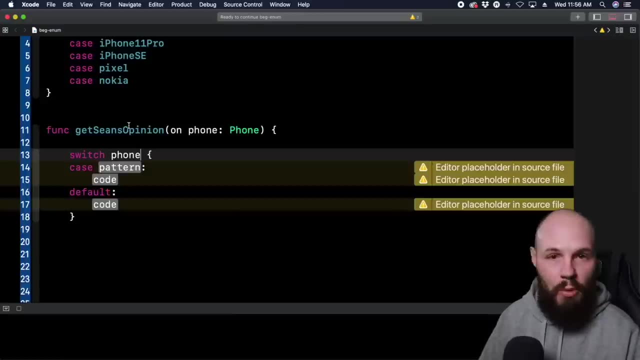 check and evaluate. so now, what a switch statement does, as you can see, is it handles the various cases again. this is why it's often paired with an enum, as you see. here we're going to do the next example where it's not paired with an enum, but again, this is common. so the first case. 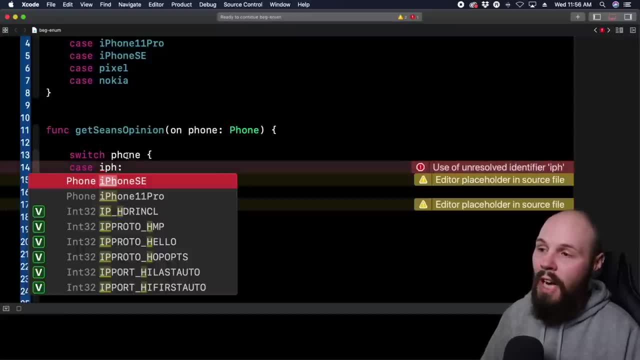 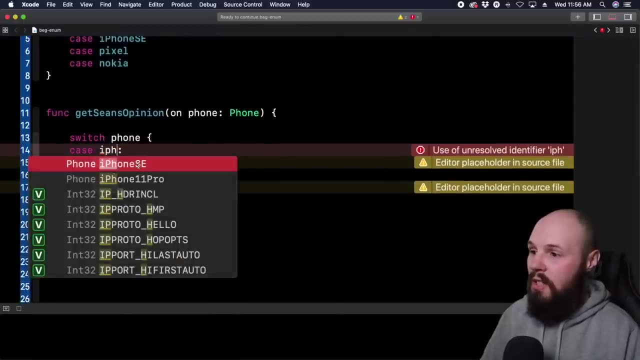 iphone and because we are switching off of a phone. that's our value. it knows that it is of type phone and it knows that it has four cases, so that's why it is giving me these cases here. so we're going to iphone 11 pro first, and now the code. this is what you want to execute whenever it's. 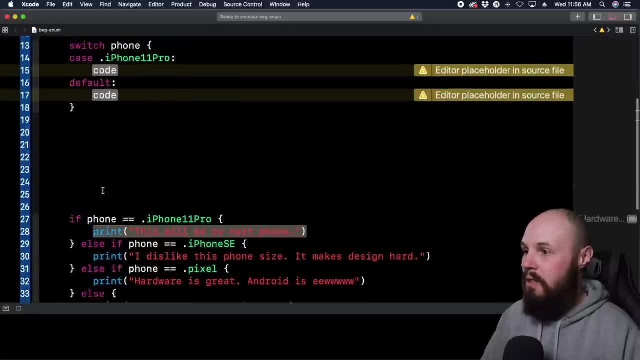 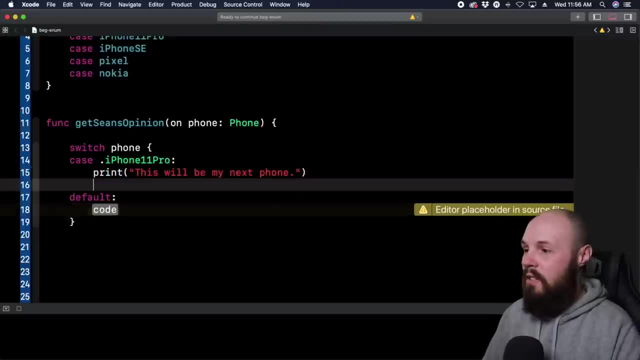 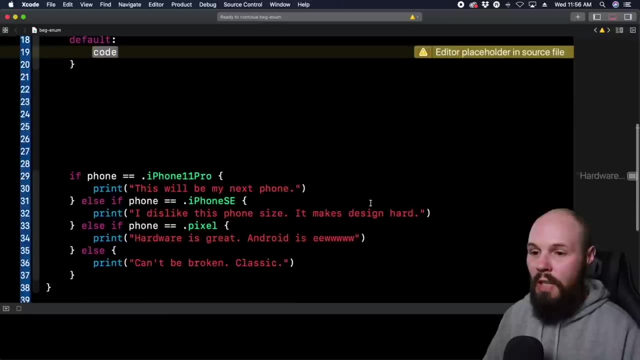 this case. so in this case we're going to copy and paste this print statement, because it's the same paste that there and that's our case for iphone 11 pro, and then now we just add the rest of the cases. so case dot- iphone se- colon. at the end on the next line we put the code again. we're just. 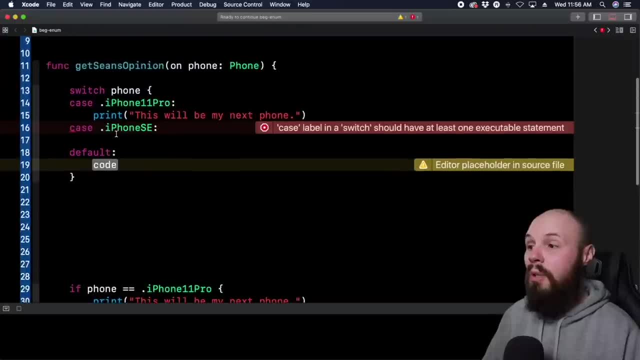 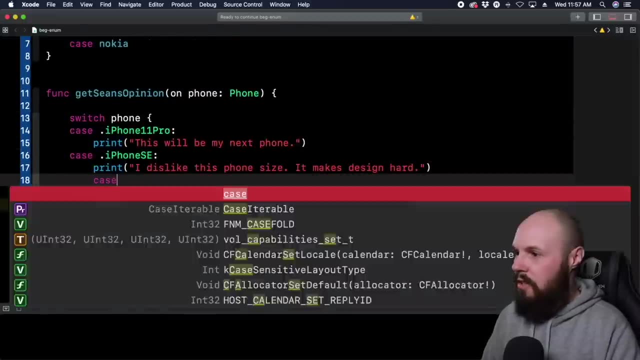 going to copy and paste this string. so, like i said, it's very, very similar to this big, long, if else, statement. it's just cleaner and more readable, as you're going to see. so case dot, pixel, colon, and then on the next line is whatever code you want to execute. now we're 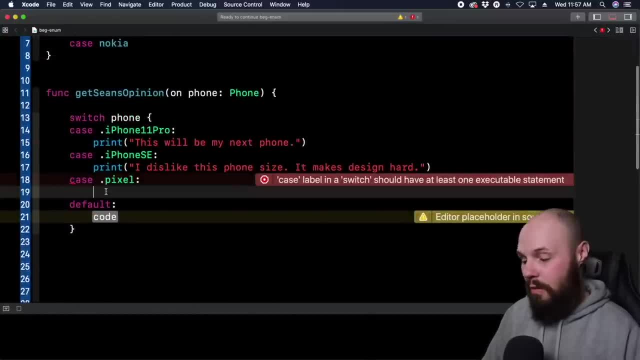 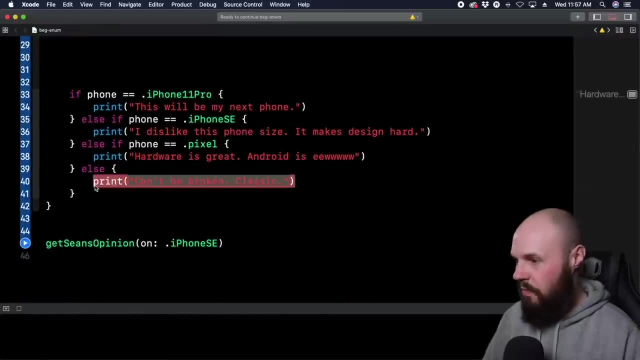 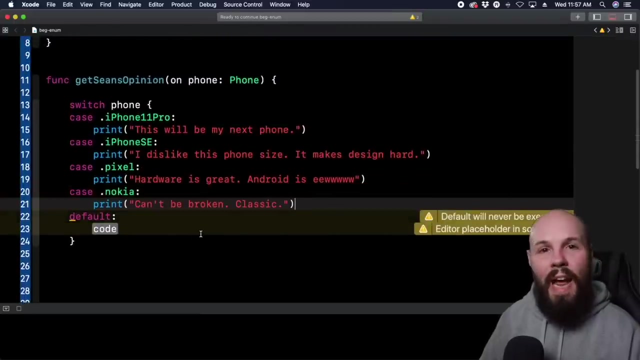 only doing a print statement, but you know this could be a whole batch of code. and then our last case is the dot, nokia, colon next line, and then the last print statement here now with um, uh, with switch statements. they have to handle every single case. now, when you declare your own enum, you know. 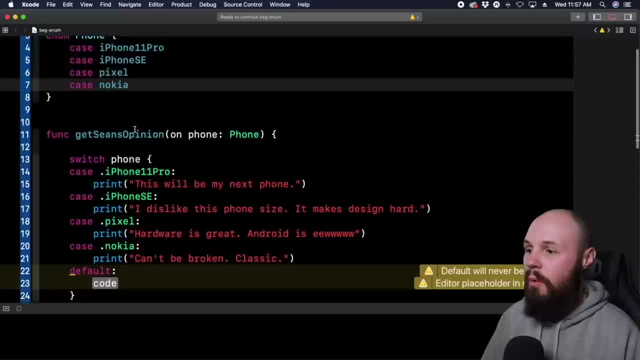 i only have four cases right, so there's not some random case. so we don't need this default because we have all uh case, love or case typically all the cas, and you're a genuine one, so it's up to you to case. number five becomes the case number once notice shift and process. ring up sequence at the. 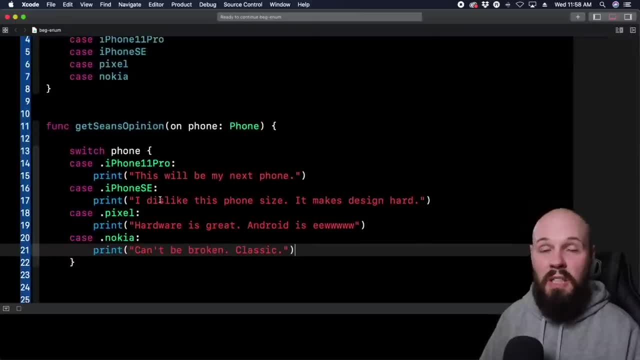 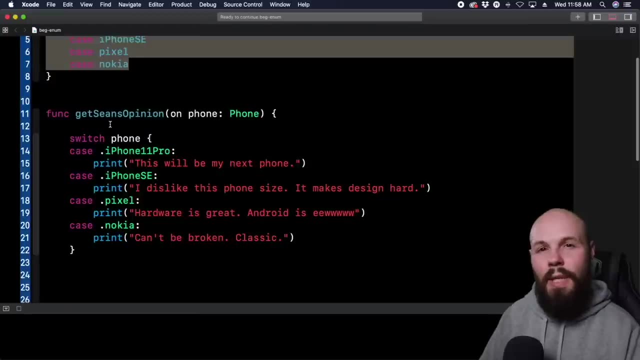 cases handled, you'll see an error. sometimes it says you know switch must be exhaustive. that means you have to handle all cases. so in this case we have four explicit phones, but let's say we didn't actually you know what. i'm going to save that for the next example, because we're actually not going. 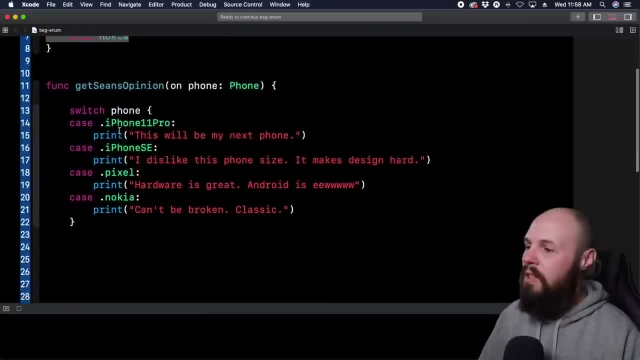 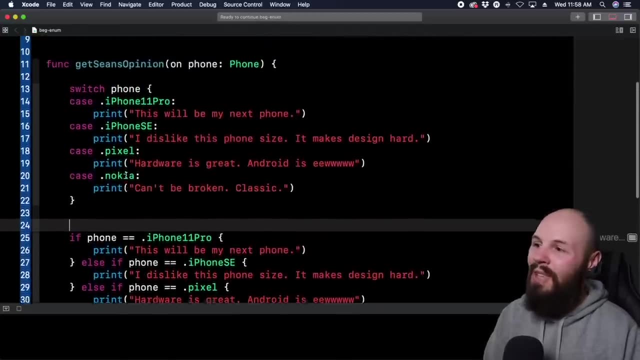 to be able to exhaust all cases. so put a pin in that. but let's put these up here. let's delete some space here again. you can see that the if statement and the switch are very similar, but look how cleaner the switch is. you can be like: hey, when it's iphone 11 pro, do this when it's the. 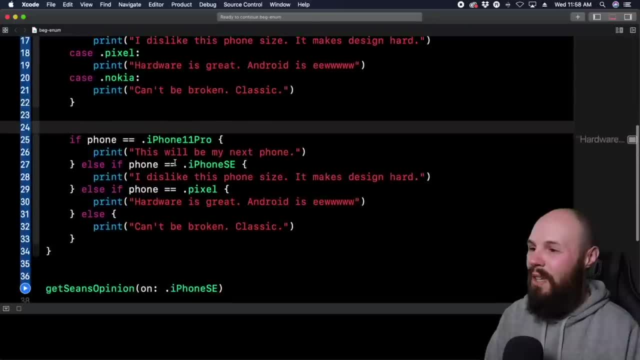 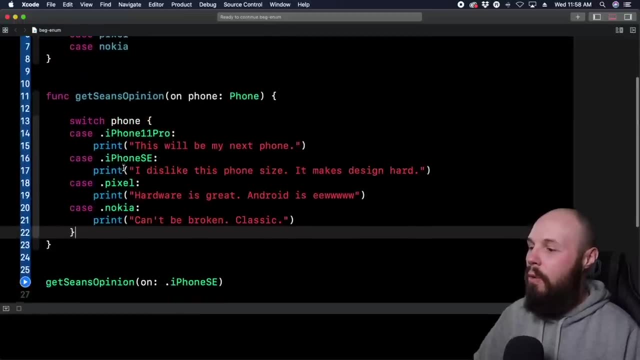 iphone se do this when it's the pixel do this, um, whereas the it's just a little more, it's just a little more cleaner. so we're going to delete that, clean this up a bit, um, and then now we'll run it. so get sean's opinion on iphone se. what it does is it passes in the phone the switch statement. 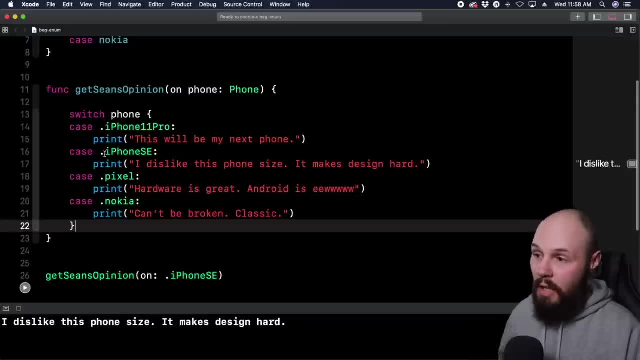 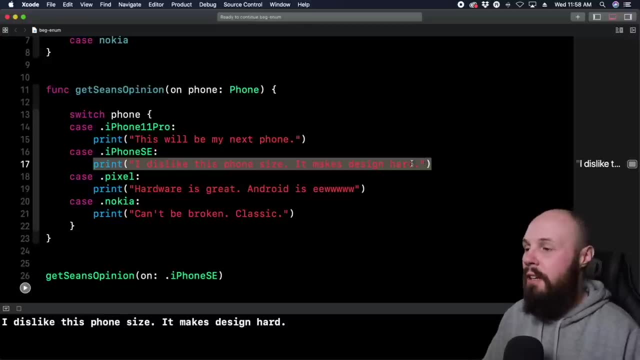 says: okay, i got a phone. which one is it? it's the iphone se. okay, cool. execute this code in the iphone se case, which, in this case, is a print statement that says: i dislike this phone size. it makes design hard, so that's how you use a switch statement paired with an. 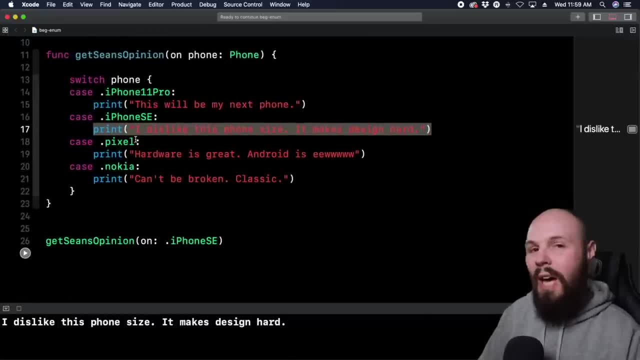 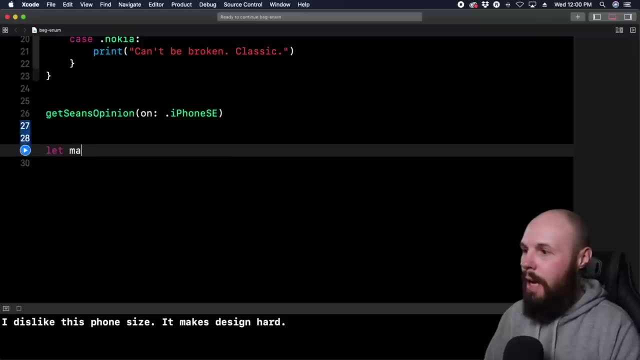 email. let's talk about a switch statement. uh, on its own, without an enum, all right. so down here we're going to create like a little ranking system. if you're, you know, ranking up in a video game or something, so let match making rank equal and we'll say five thousand for now. so, uh, let's actually 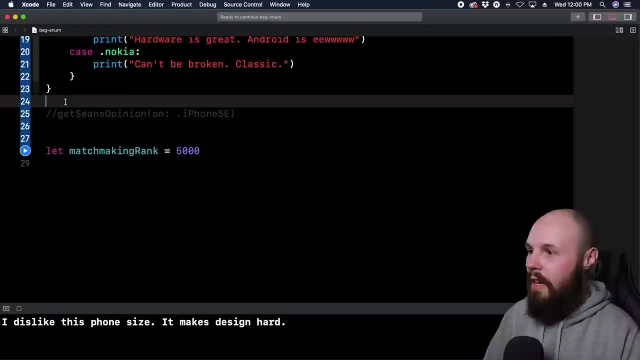 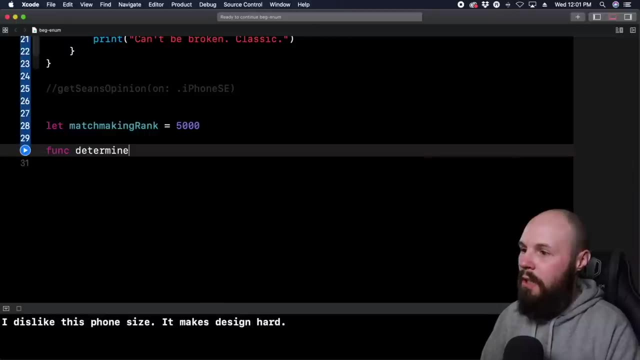 comment this out so we don't get any confusing print statements there. so that means we're not actually going to run that function. so let's create, uh, our function here to determine our matchmaking rank. so funk, determine player league, and then you can do from again. this is the argument label and then rank is the parameter label that we're actually 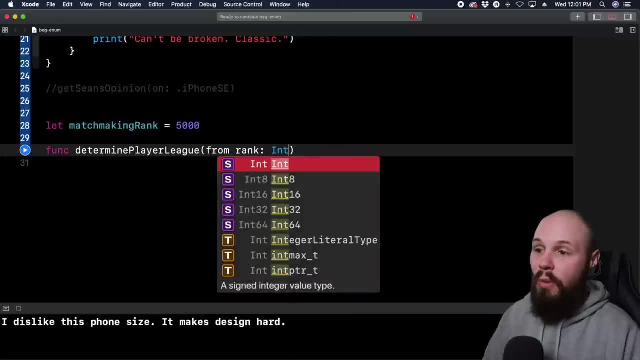 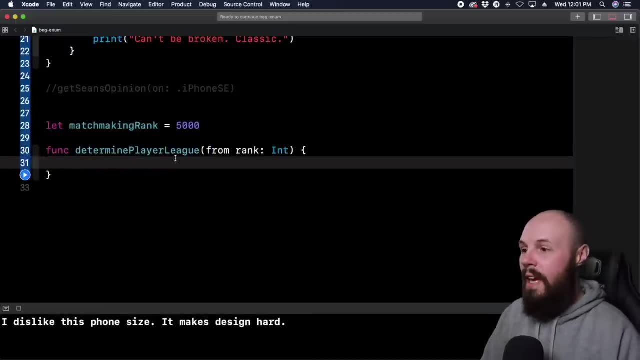 going to use in the scope and then the rank is going to be an int. that's what we're going to pass in, because that's what this is up here on line 28. that's an int. get our open and close curly braces for the scope of our function and now we do a switch statement based on the rank that we're 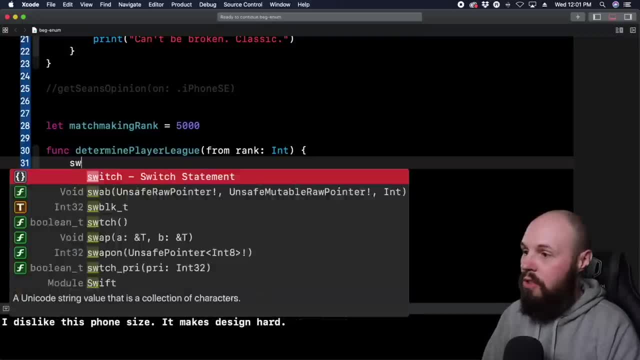 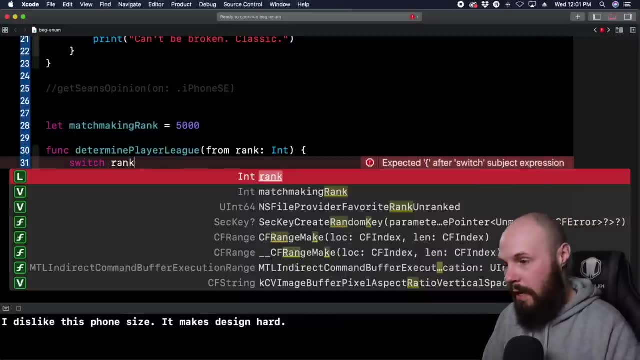 passing in an int. now here we're not paired with an enum, but we can still do switch and we want to switch off of rank, which again is our parameter label. that is an int, you can see it shows a type int and we want to have various cases. so we do case zero and return. we're going to put the code. 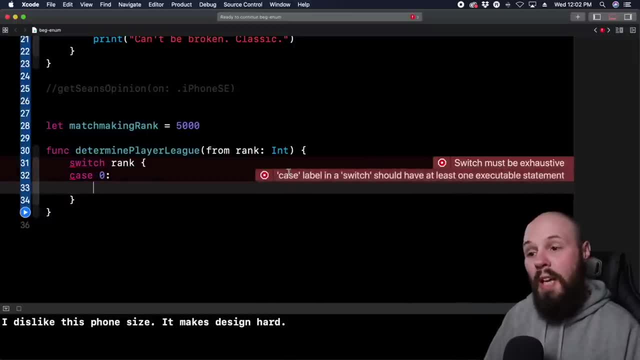 there, but you can see our error right here. that switch must be exhaustive and then also case label, and a switch should have at least one executable statement. so you have to have uh, some code in there. so let's do uh print: play the game to determine your league. so basically, this is what. 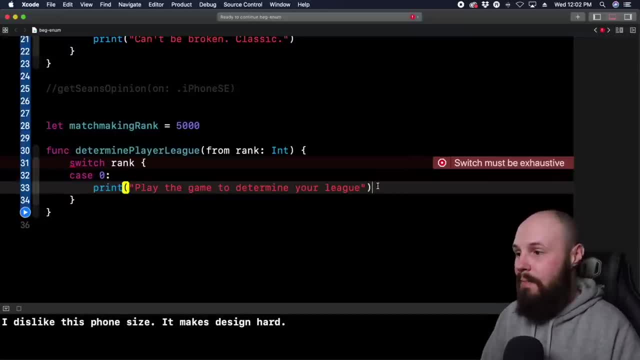 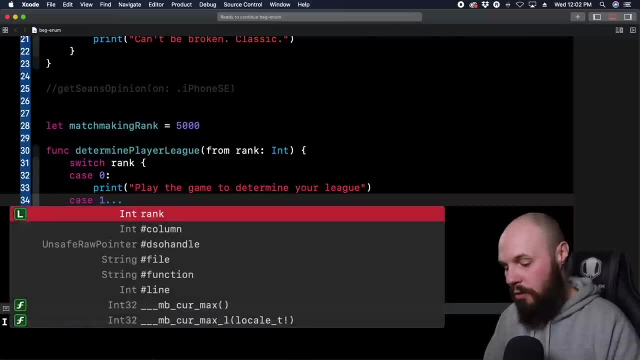 happens when our match ranking rank is zero, like we haven't played a game yet, right, so now we do case uh. here's where ranges come into play as well. so from score one dot dot dot up into uh, up into less than 50, that's our next case. now we can do print. 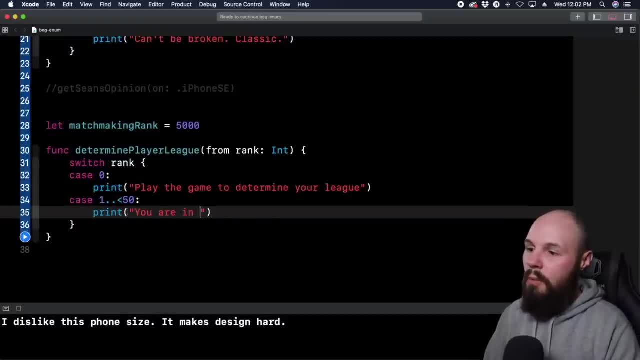 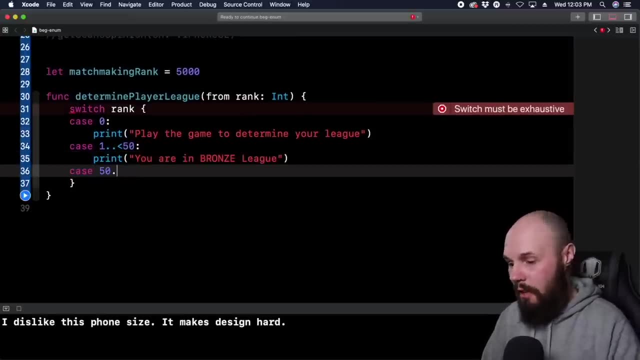 uh, you are in bronze, uh league, and then, continuing this, we can do case uh, 50, dot, dot up until 100, and let's just copy and paste this to save some time. copy paste, you are in uh, uh, silver and you can see where this is going. i'm only going to do up to gold and then the 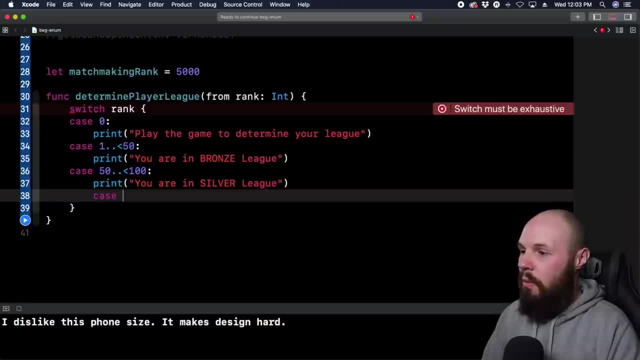 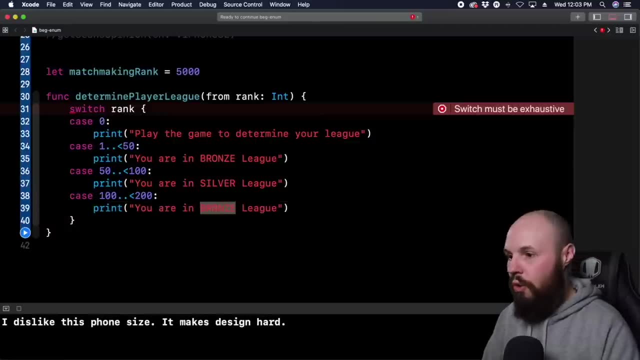 default case. we'll talk about that. so case: uh, 100, dot, dot, uh, up until 200, paste that you are in gold league. so again, the way this switch works- and we'll get to this exhaustive in the default case in a second: uh, we're passing in the rank and then it's going to switch off the rank if you are zero. 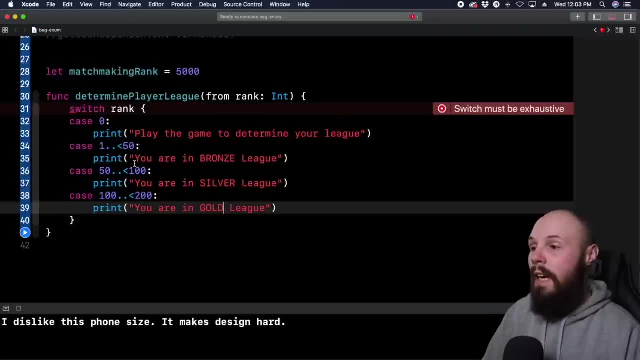 you're going to say determine, uh, play a game to determine your league and then, if your int falls in one of these ranges- again, we got a good review on how to use ranges- it'll print the appropriate message. now you'll notice it only goes up until 200. well, the switch must be exhaustive, meaning it has to handle every possible. 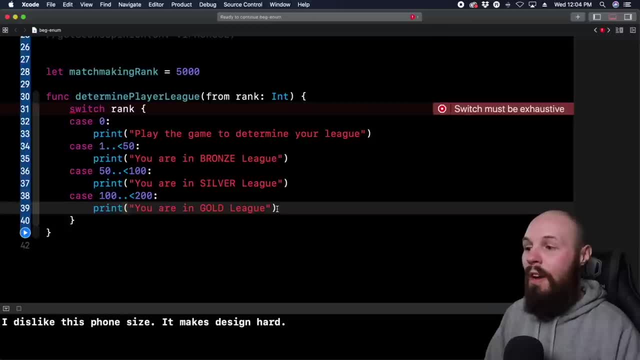 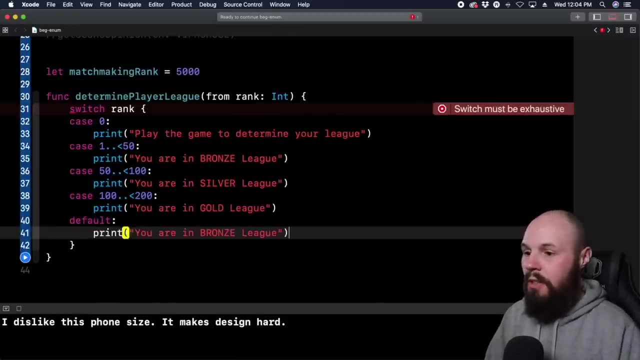 case. so in order to do that, uh, when you don't have, like, an enum that has a set number of cases, you do default. this is basically your catch-all. so the default we're going to do print. uh, you are in a league of your your own. you are too good. 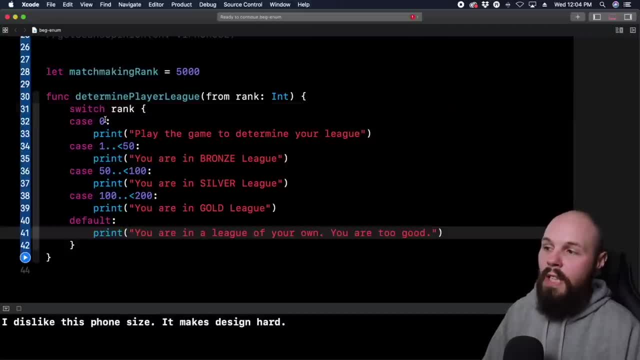 meaning like you're in a league of your own. you are too good. you are in a league of your own. you are too good, like you. you're above 200, right, because we're handling everything else well. we're not handling negative numbers actually. uh, so maybe this is the wrong message. let's play. you're in a league of. 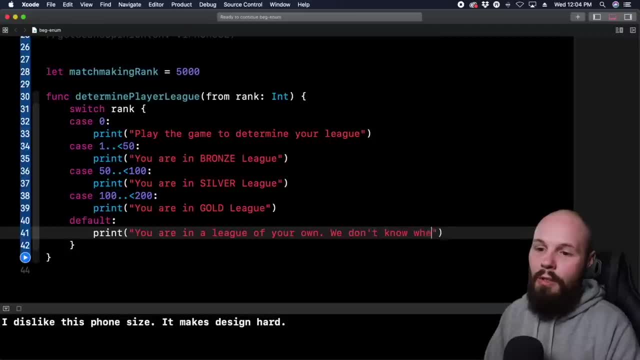 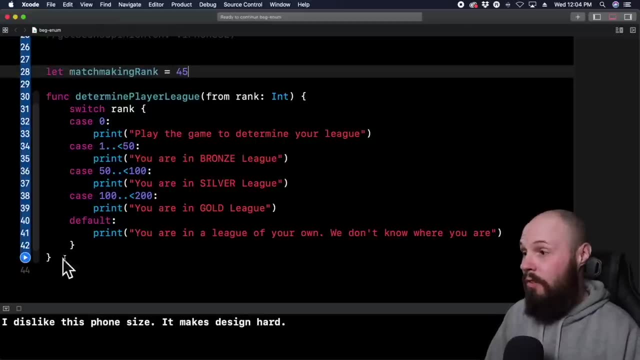 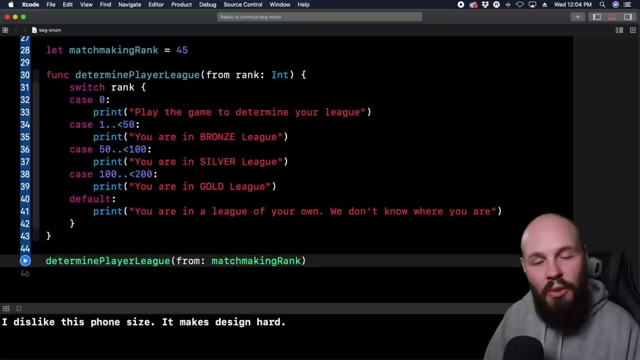 your own. uh, we don't know where you are, so let's test this out. let's pass in a 45. that should put us in bronze. uh, we actually have to call the function. sometimes i forget to do that. so determine player league from uh. match making rank. again the the readability of swift determine. 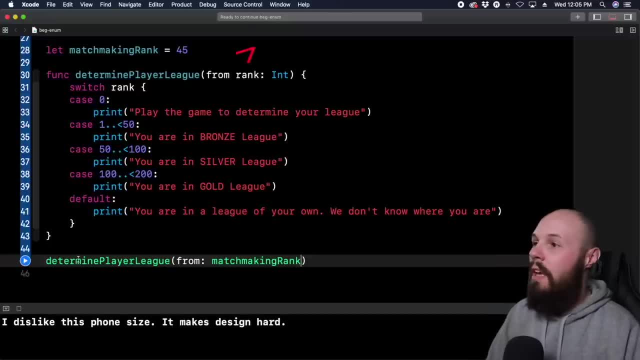 player league from match making rank. so good, so good, and our matchmaking rank is up here, uh, and it's equal to 45. i just changed that. so we should go into, uh, bronze league. let's run it to test it. yep, you are in bronze league, uh one. 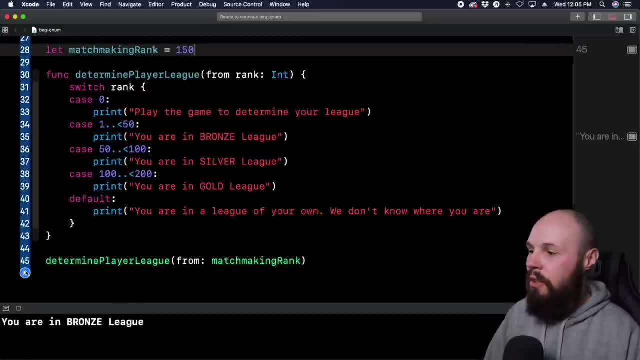 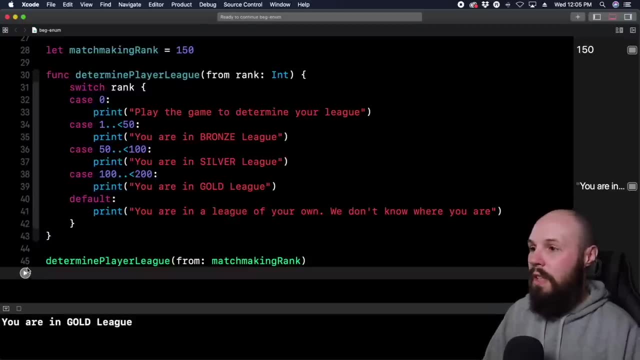 more test or two more tests, call it 150. that should put us in gold and you can see. if you're making a video game and you want to assign a player, certain leagues like you can do something like this: uh, you are in gold league. now let's test out our default case. so let's do one and a lot of. 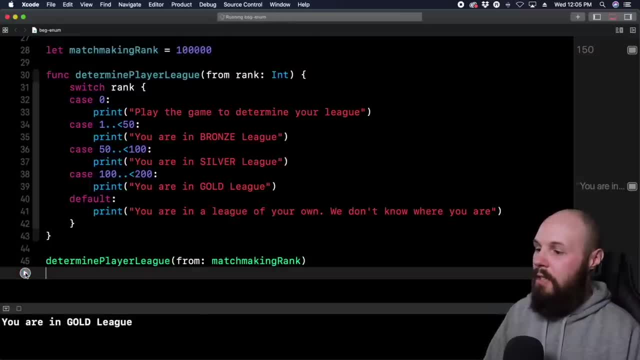 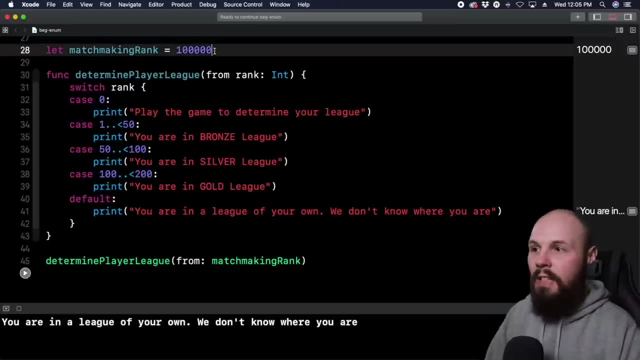 zeros right there. i don't even know how. what is that? ten thousand hundred thousand? uh, it says you're in a league of your own. we don't know where you are. that's because it went into our default case, which was kind of our catch-all. and again, negative numbers, right you? 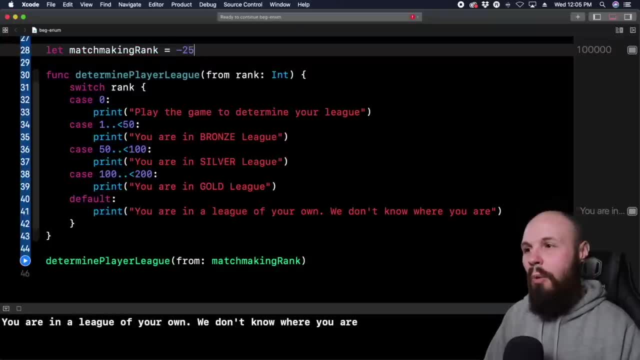 wouldn't think matchmaking could have negative numbers. but this is kind of the point of programming: is handling the edge cases right? so, uh, run it again. it's going to say again you're in a league of your own, we don't know where you are because again it doesn't fall into any of our cases. so 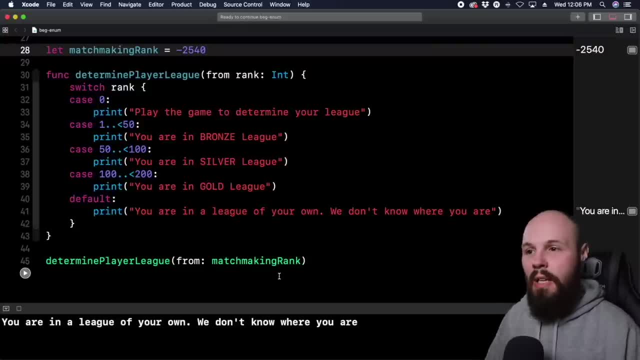 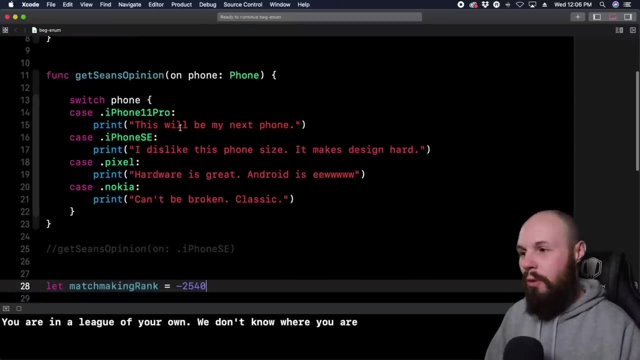 the default is the catch-all. so that's the basics of switch statement and again, to put it super simply, if you just remember this, it's just a neater, cleaner way to write a big long if else else- if statement right that we saw up here previously. with this switch statement right, this just looks a lot cleaner, it's more straightforward. 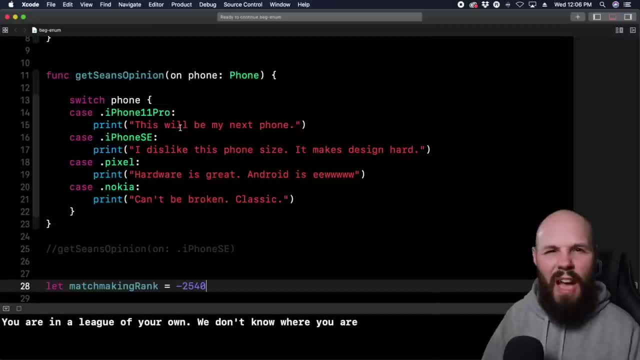 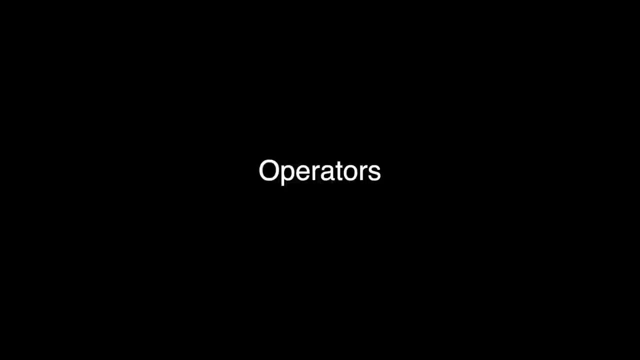 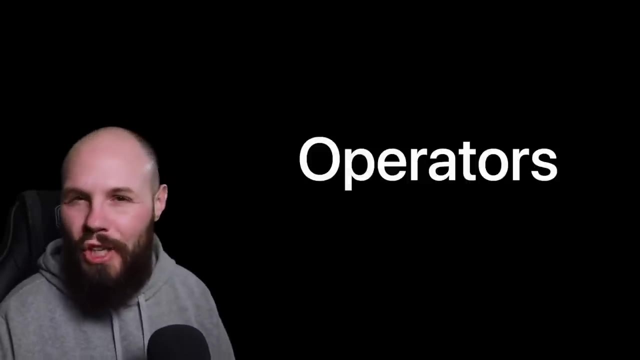 easier to read, so utilize the switch statement if you see yourself having that big. if else, you know mess. you got going on there all right on to the next video. let's switch gears a little bit and talk about operators. in swift now, operators allow you to check, change and combine values. 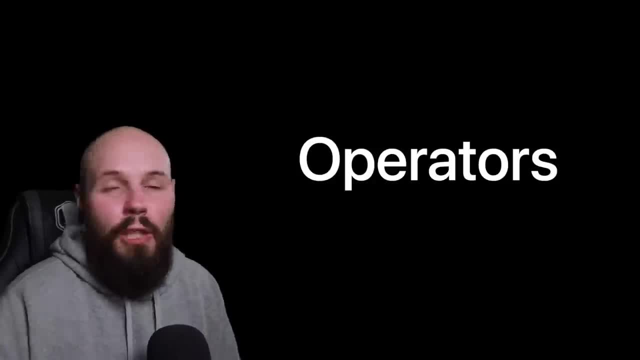 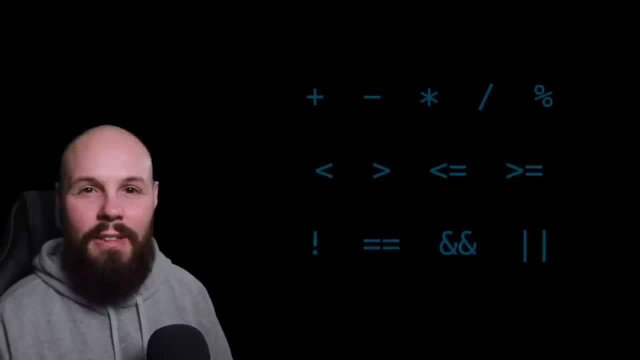 um, that may sound a little complicated, but think about it like, like you're already familiar with the term, right, operators are like math, you know: addition, subtraction, multiplication, division. uh, think of them like that and actually that's the example we're going to start with. is those basic? 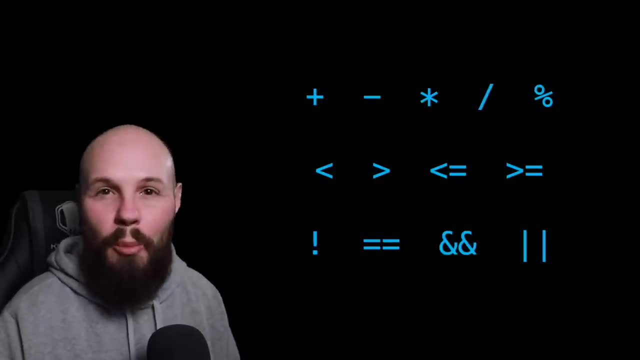 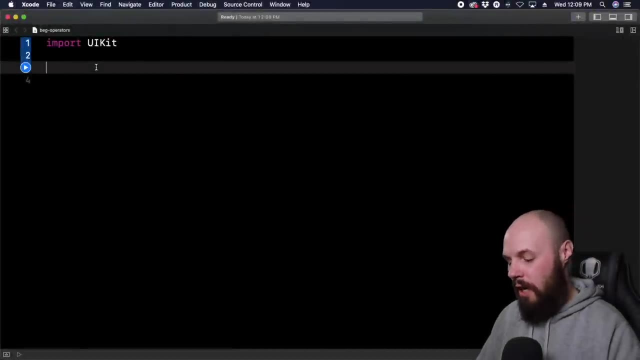 math examples, uh, but as you can see, there's many, many more operators and hopefully you can see how useful they are after this video. all right, here i am in a blank playground, as always. feel free to create that yourself. let's create two values here, so let value one equal- i don't know whatever. 55. 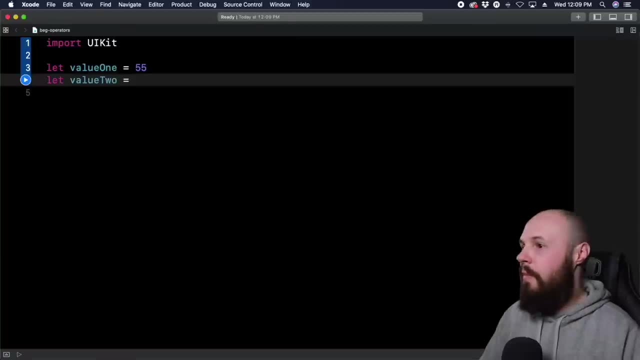 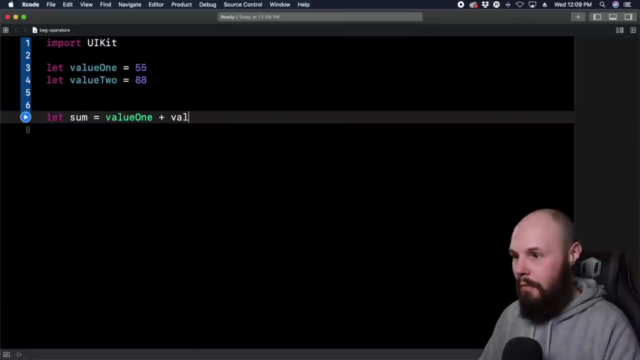 let value two equal 88, um. so now here we can do: let sum equal value one plus value two. all right, we're back to back to first grade. um. simple addition with the plus symbol. all right, hopefully i don't have to drill that point home now, that is the you know addition operator, and then now this operator. 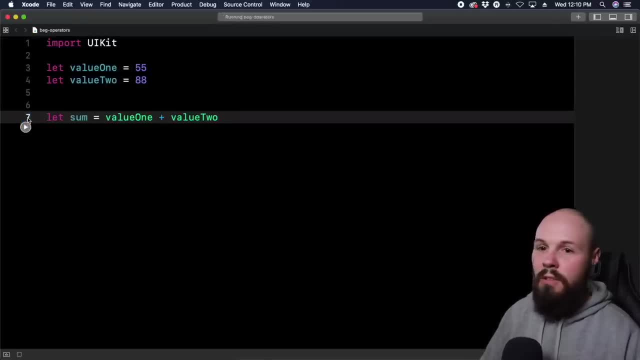 well, let's actually uh, run it so you can see the sum. to check it: 143. uh, now we can do value one minus- again very basic math. but we're going to run through this real quick now. it's negative 33, right 55 minus 88. negative 33 checks out, and to do multiplication you do the asterisks or shift. 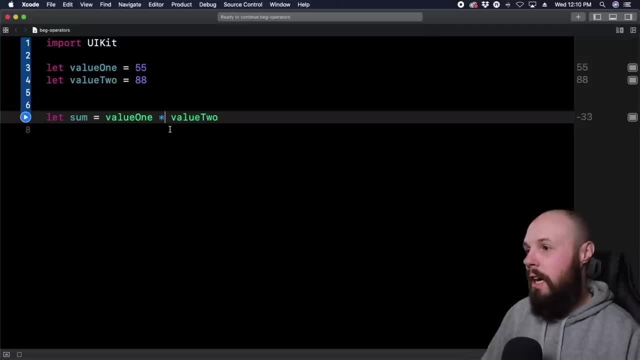 eight, uh, for the star. that is multiplication here. uh, so i don't know what 55 times 88 is, but we're about to find out about 4840.. now, that was all smooth sailing. now's where it gets a little tricky, um, because division here, uh, we're going to do 55 divided by 88, which, as you can see, 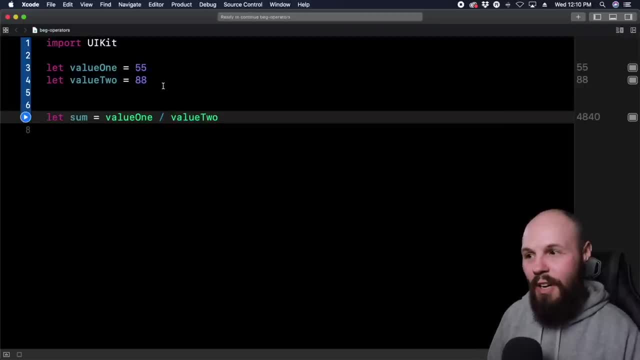 which, as you can tell, that should be less than one, that should be a fraction. but watch what happens and we'll explain this. so let's run this. so there's going to be 55 divided by 88.. zero, that's not right. here's why. so, via type inference, these are ints. so a property of ints is int is always. 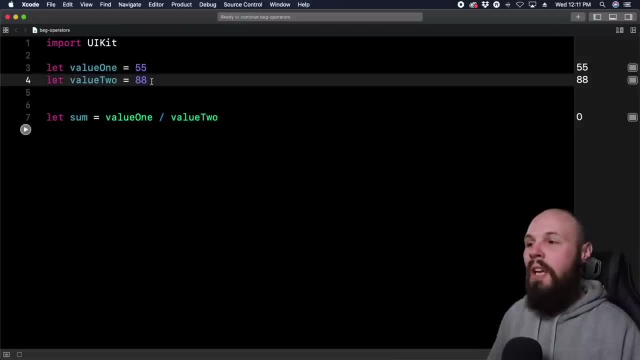 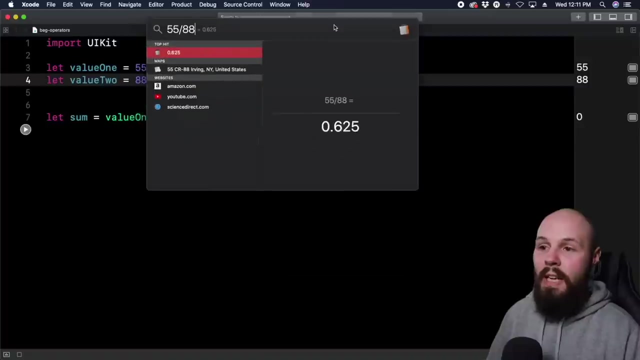 a whole number and int can't be a fraction. so the way swift handles ints when it's a fraction is it just literally cuts off the decimals, right? so this should normally be? i don't know. let's do it: 55 divided by 88.. this should be 0.625. so what it does, uh, is like i said, it just drops the decimals. 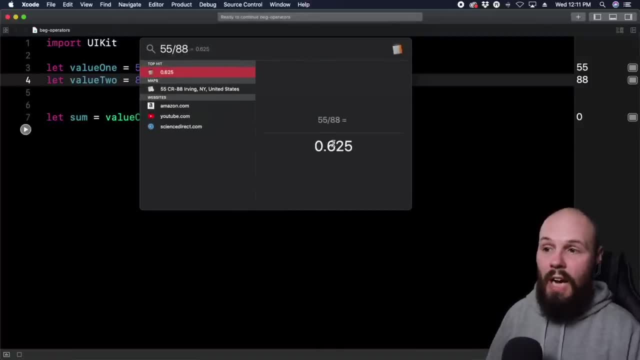 so that's going to be zero. now, if this was 1.625, it would drop the decimals, so it would show up one again. this is only when you're using ints versus ints, because an int is a whole number, no matter what. and the key thing to remember, it doesn't round up. it doesn't round down, it just drops. 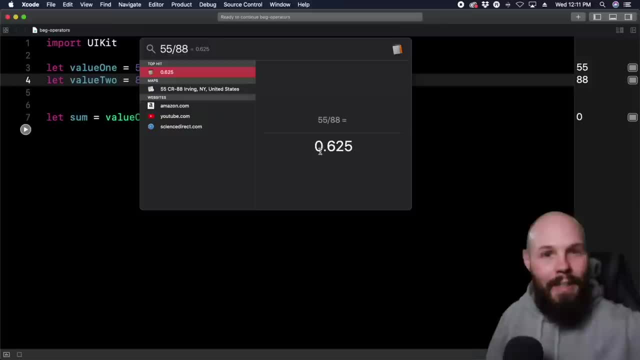 the decimal. so even if this was one point- nine, nine, nine, nine, nine, nine- it wouldn't be two, it would be one- drops the decimals. so when you're dealing with ints, just remember that. uh, when it comes time to use division, so if you're using division and you want percentages, you have to. 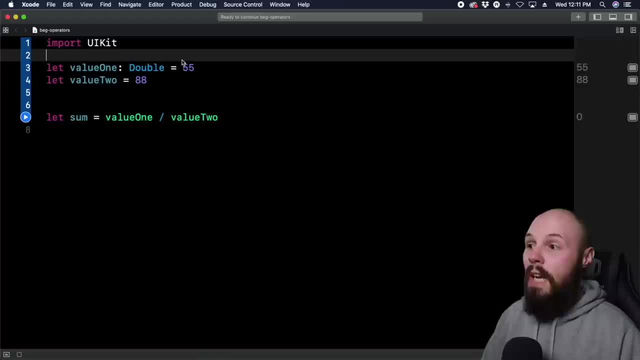 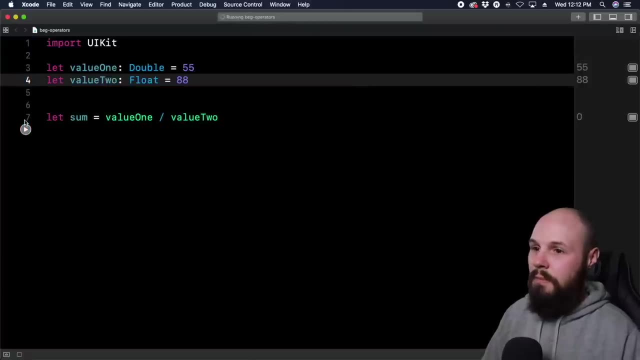 make these floats or doubles, you know. whichever one you two choose now, they have to be the same, right? i can't divide a double in a float, right? you're gonna? you're gonna see xcode's gonna yell at me. binary operator. the division sign cannot be applied between operands of double and float. 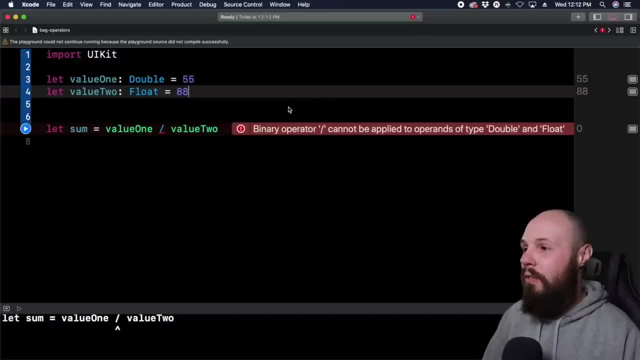 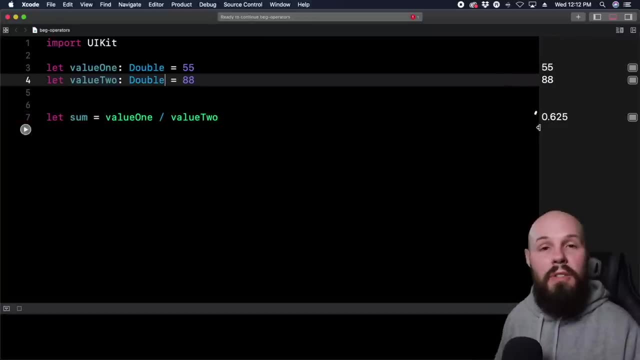 so when you're adding and subtracting they have to be the same type. so if i go back and make this a double now it's the same type. i'm not going to get that error. and then we get that 0.625 number that you saw me do in spotlight. so again, math was simple up until we got to division. key thing to. 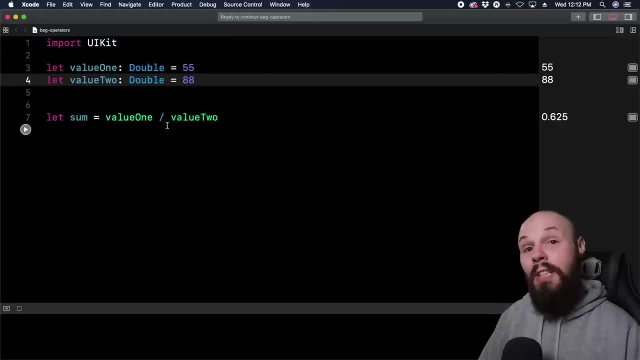 remember an int is always going to be a whole number and it's not going to round up or down, it's just going to drop the decimal. so i bet that'll still get you in trouble, even though i kind of reiterated that happens to all of us. so those are some basic math operators. 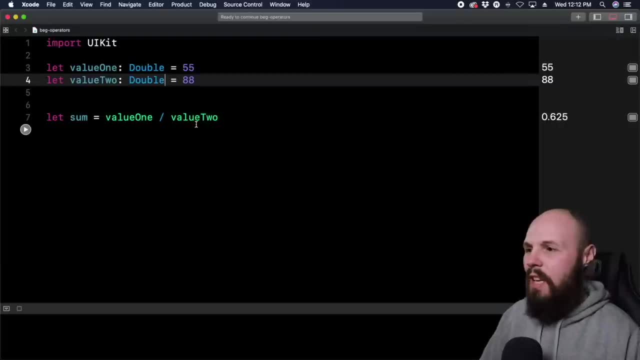 one more that is unique to programming, or at least i haven't seen it outside of programming- programming, and that's the modulo operator. so to show you that, let's go back to ints here. uh, so to do that, we're just going to get rid of the declared type. so this is automatically. 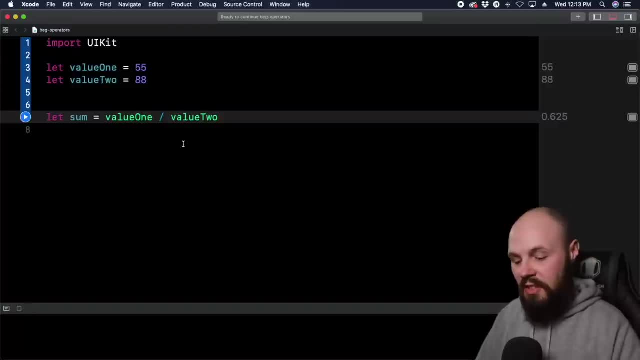 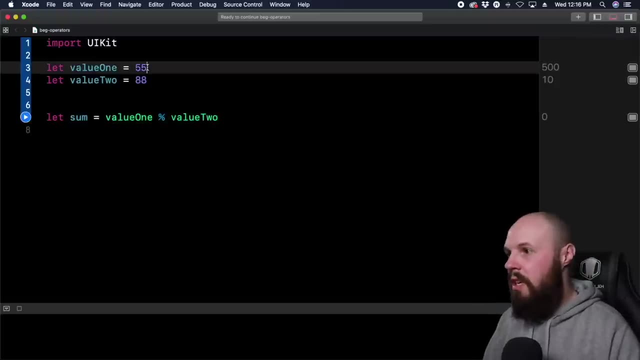 going to make those uh ints. now what this does is it's similar to division only because it deals with remainders and the modulo operator is a percentage. so let's change these values to make a little bit more sense. so uh say a value, one is uh 100. so how many times does 88 go into 100? 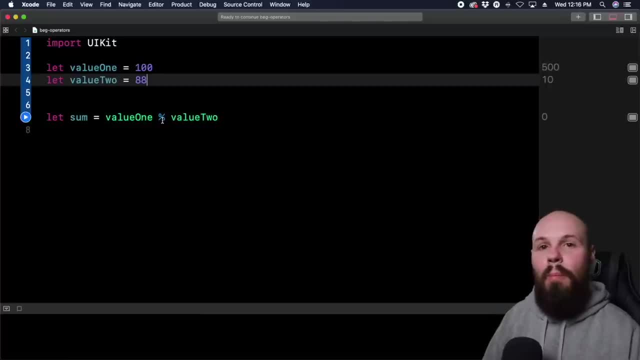 is what modulo says and what it does is it gives you the remainder. so 88 goes into 100 one time, uh, but it also has a remainder of 12, right? so? because 100 minus 88 is 99.. if you remember back to very early elementary school math, you would say 1 with 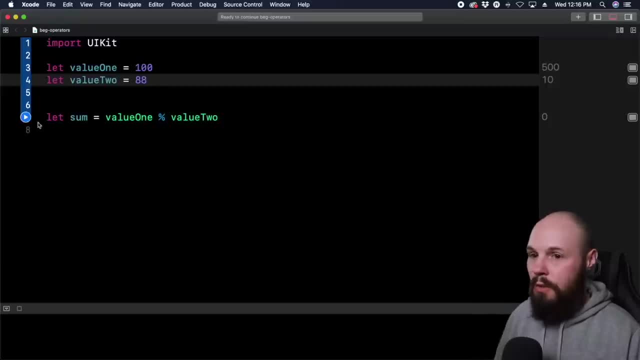 the remainder of 12 is how many times 88 goes into 100.. so let's run it and the modulo here will equal 12, as you can see. so it's similar to division, except you're only getting the remainder right. that's all it spits out. so now make it a thousand and make this whatever. uh, 881, uh, so it's. 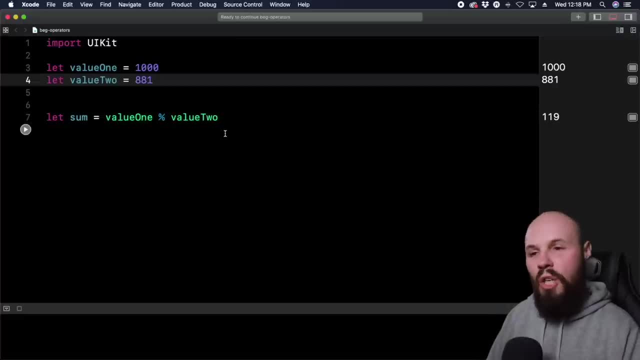 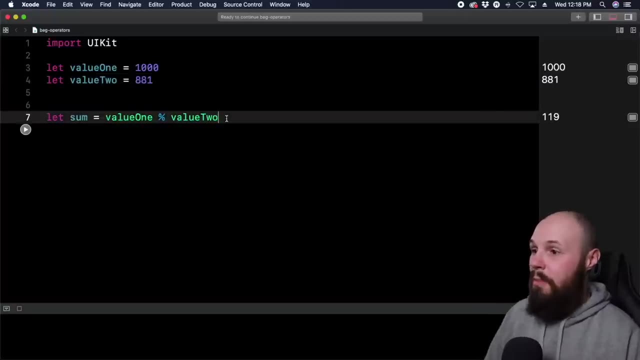 going one with a modulo of 119.. so that's modulo, and again, that will give you the remainder of how many times one value goes into another. uh, now let's start talking about some equal signs. you know what? i'm just going to leave this up because we're already here. so, and i've mentioned this in 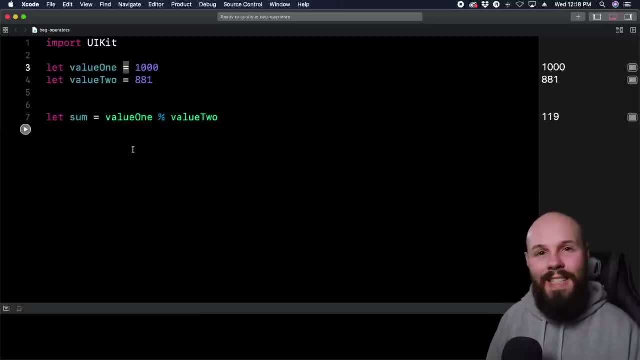 a previous video how one equal sign is considered an assignment operator. right, we're assigning 1000 to value one. we're assigning uh 881 to value two. here we're assigning you know the. well, some apologies, sum was probably the the wrong variable name for the. you know multiplication and all that. 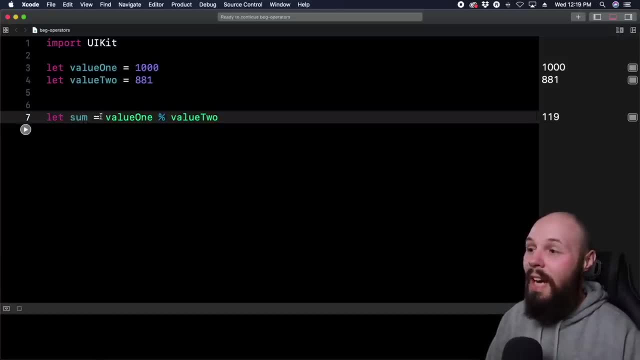 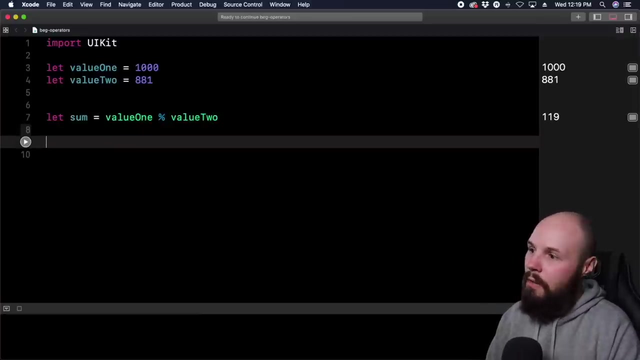 stuff, um, but sum is: uh, we're assigning the modulo, which is 119, to the variable sum because of one equal sign. right, we've done this a lot. um, now compare that to two equal signs. that is where you're saying: is this equal to that? so we're going to basically say: value, one equals equals value. 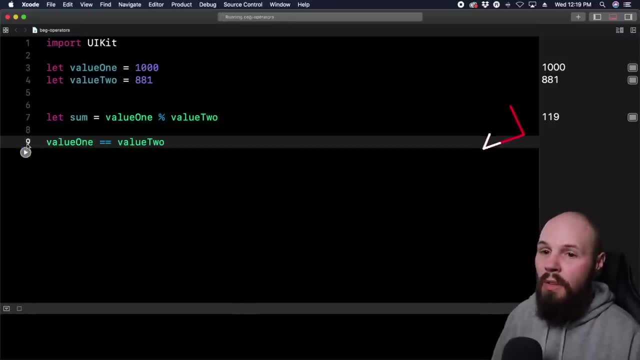 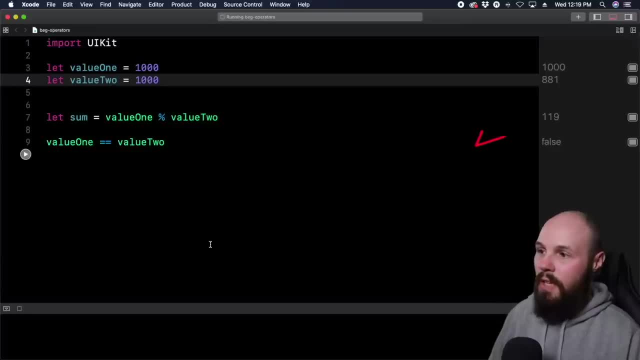 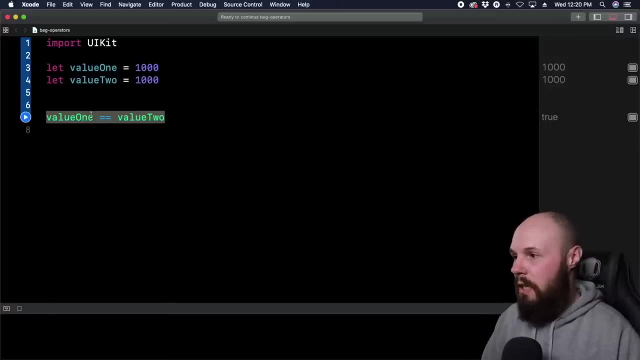 them equal and run that again. now we get a true because they are equal. let's get rid of this to avoid confusion. so, before we use this in our if statement, right, so let's, uh, let's do that. if value one equals value two, uh, print they are equal, run it and there you go. we've done this. 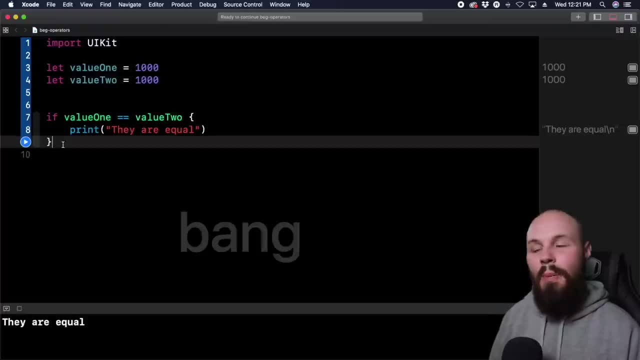 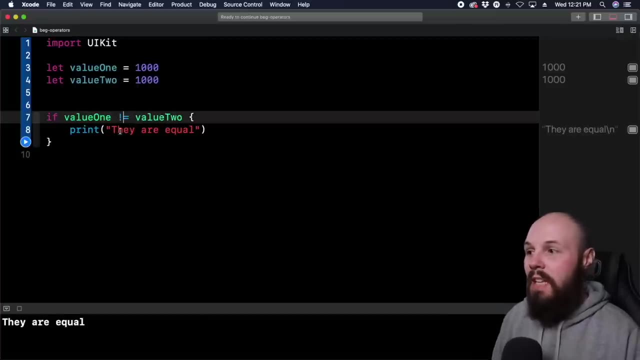 before. hopefully this is review. they are equal, so it happens. now let's talk about the bang operator. uh, or an exclamation point. so instead of equals equals, if we put an exclamation point here, what this is saying is: if value one is not equal to value two, now we want to say they are not equal. 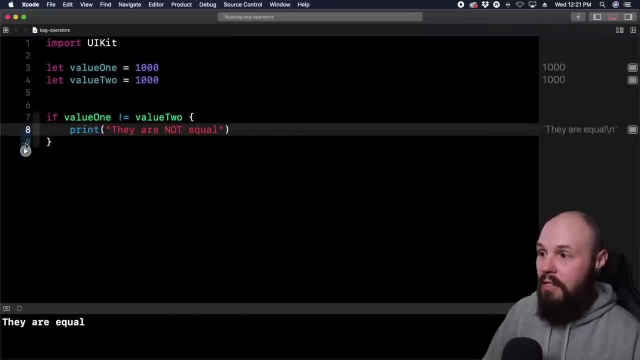 but this isn't going to run, this isn't going to execute because they are equal, right, thousand equals a thousand, so we're going to see nothing print down here. but if we change this, you know a thousand and ten, it is going to, uh, go into the scope. they are not equal, because this means not. 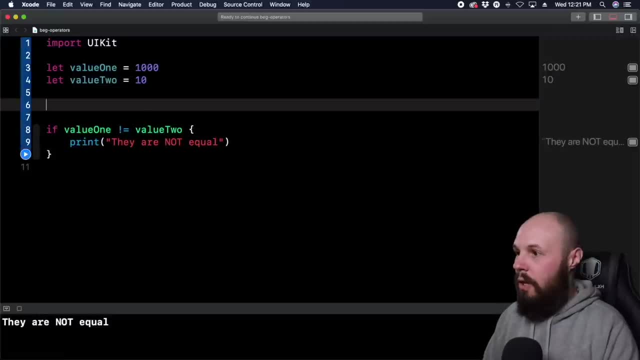 equal to now. another version of the bang here is back to our uh. var is the value one equals one. so is dark mode on: equals true. right, that equals true. so another thing we can do here is remember we've did this before- value uh is dark mode on this is going to uh evaluate to true uh. 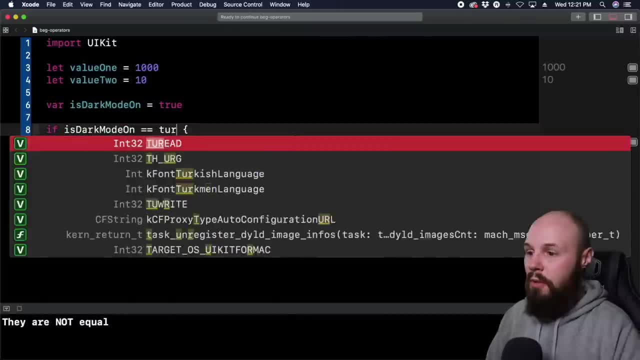 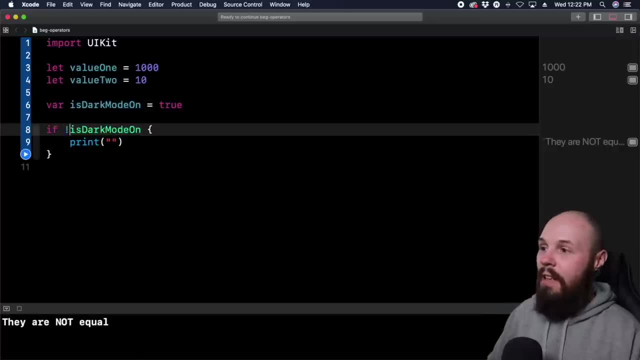 automatically. i don't have to do equals, equals true here. right xcode is smart enough to uh handle the boolean that it defaults to true. so now, if i put the bang operator in front of that, that is now saying, if dark mode is on, equals false um. so we're going to say, uh, it's. 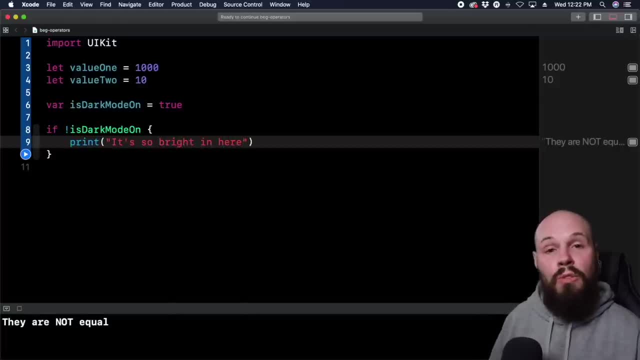 so bright in here? because is dark mode on equals false? that means it's not dark mode, so it's so bright. so, uh, is dark mode equals true? so that means this is not going to execute, right, because we want this to be false. that's what the bang operator tells us now, when i flip this to false. 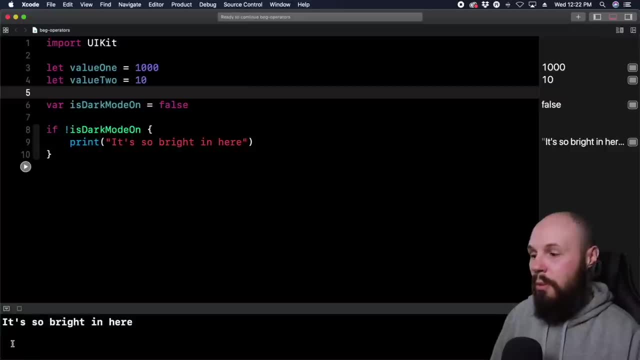 now it should execute? uh, because it is false, so it's so bright in here. okay, that's what's known as the bang operator. it's meant for it like not being equal to now. one thing we're going to get to in a future video is optionals, and one way to unwrap optionals is to put 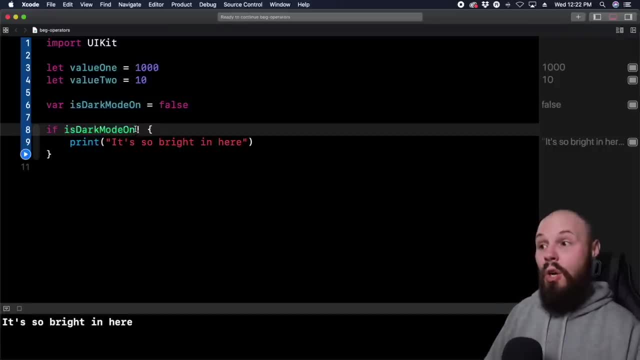 an exclamation point at the end, right, so uh don't get too confused. the, the bang operator at the beginning, is what flips the uh, the conditional, you know, or the boolean to false. uh, the bang operator at the end is for unwrapping, optional. so just want to clear that up and again. more on unwrapping: 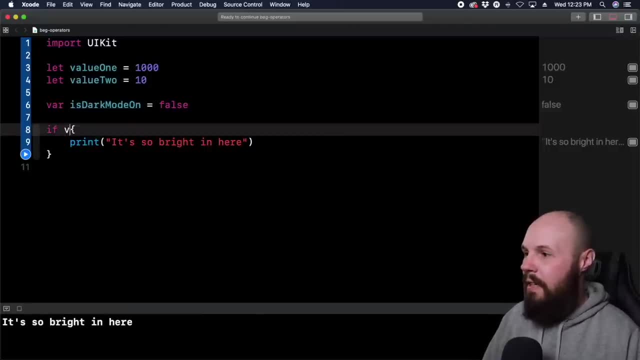 optionals later now let's go back to the example uh we had of uh, value one equals equals value two. real quick, while we're here, we, you can do the uh greater than. if value one is greater than value two, do something. uh, you can do less than. you can also do the. you know less than or equal to that works. 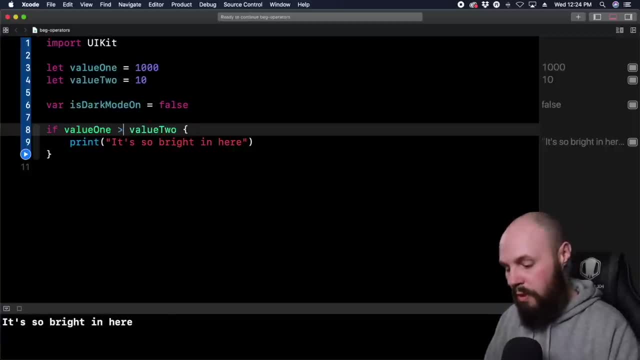 uh, or you can also do the greater than or equal to- oops, right, and that means if it's bigger or equal, to then execute again. those are basic math principles that, hopefully, you learned when you were just a child. but now let's talk about uh, the or and and operator, and i'll show you that. so this: 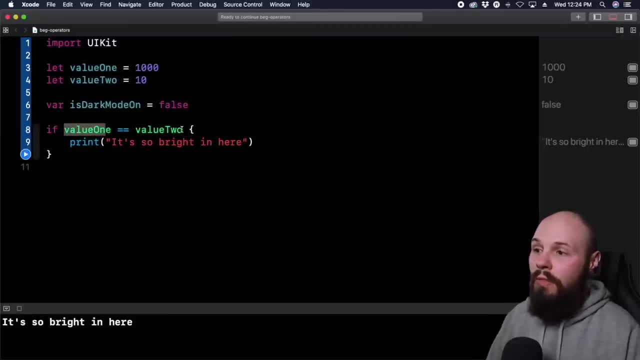 is auku looking for, though, just as a. we don't want to use basic math principles, right? so we would say, if value one is equal to value two, and you can do, and uh, is dark mode on equals, true, so this is a way to handle like two scenarios. so we only want to execute this code. uh say dark mode, yes, and 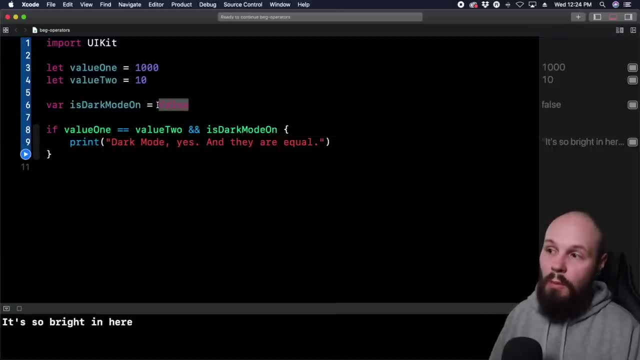 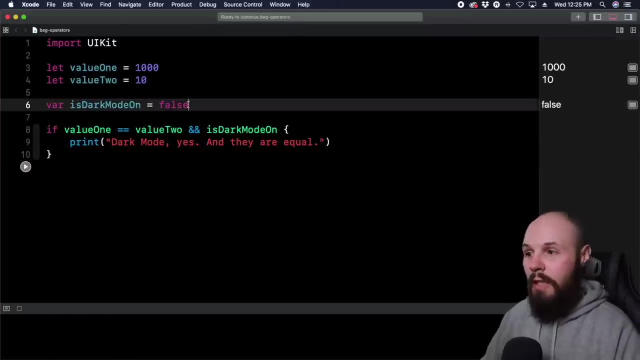 they are equal. we have isDarkModeOn is false right now, So if we run it, it's not going to execute anything, as you see down here, because isDarkModeOn is false Again when you use the, and they both have to be true, So run it. And now it's. Oops, I forgot to make these equal. 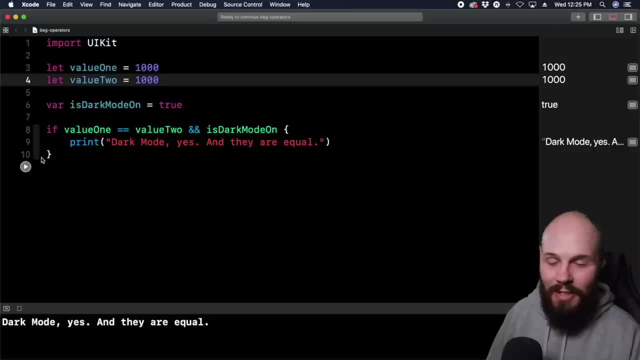 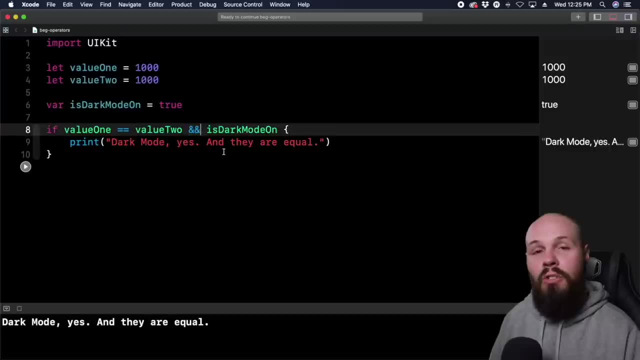 One, two. So there you go, See. now you see, they both have to execute, as I accidentally showed. Now they're both true. So dark mode, yes, and they are equal. So that is the and operator, And that is by two of the ampersands. Now the or operator is another thing you use in your 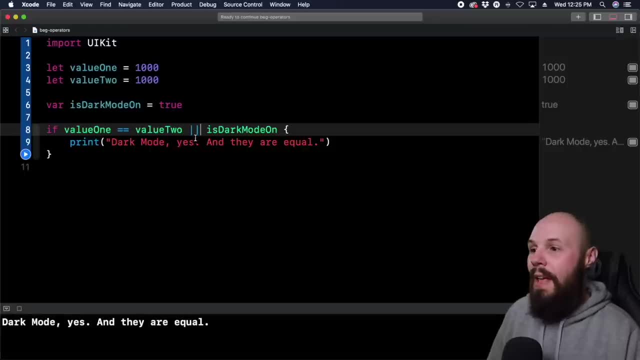 F statements or conditionals as two vertical pipes, And that means either one of these can be true- right, And was they both had to be true- or just any one or the other. It doesn't matter if it's only isDarkModeOn is true and this is not true, Like just one of them has to satisfy. 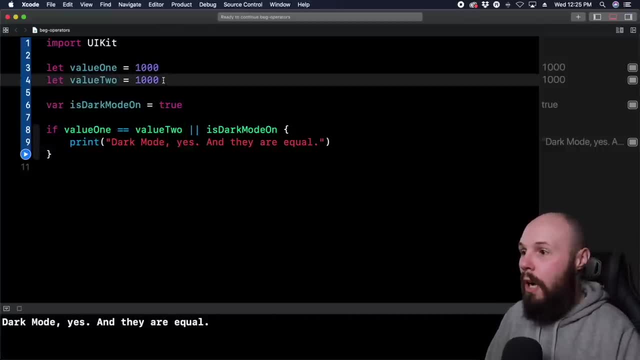 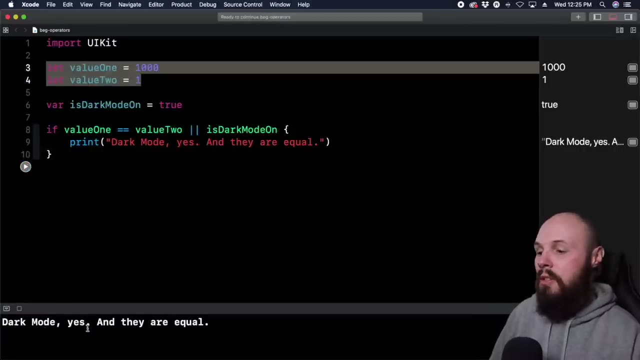 the condition and the code will execute. So here's a good example. We're going to make these not equal, but isDarkModeOn is true and the code will still execute. So you see down here: yep, dark mode yes, and they are equal. Now two more things before we. 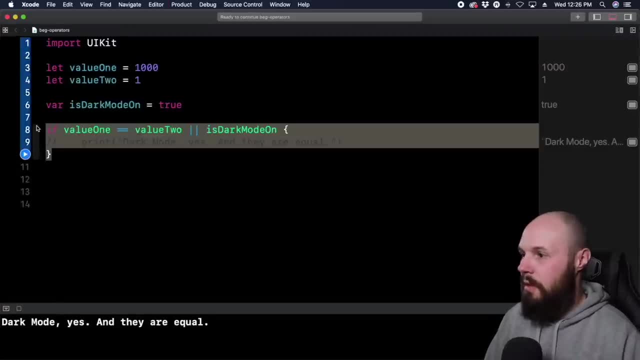 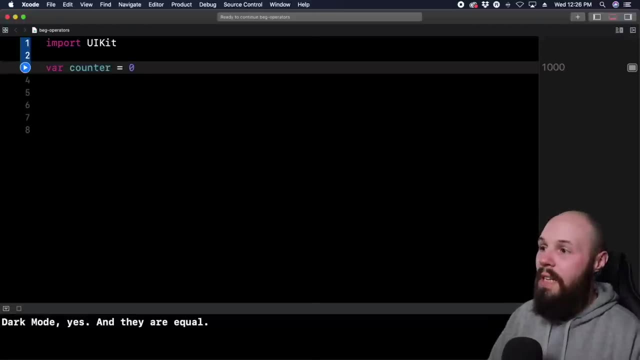 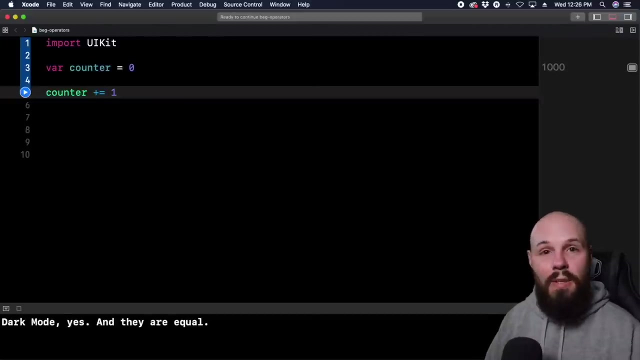 finish up the operators. Let's get rid of this code here. Let's just get rid of this altogether. You know what Let's just really clean up here? Let's do var counter equals zero. right, There's my int. that equals zero. Now we can increment this. We can do counter plus equals one, So that 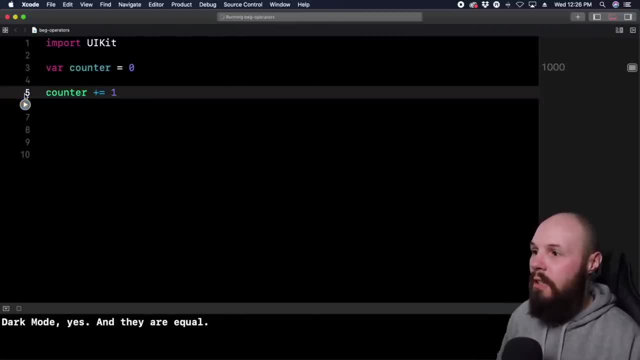 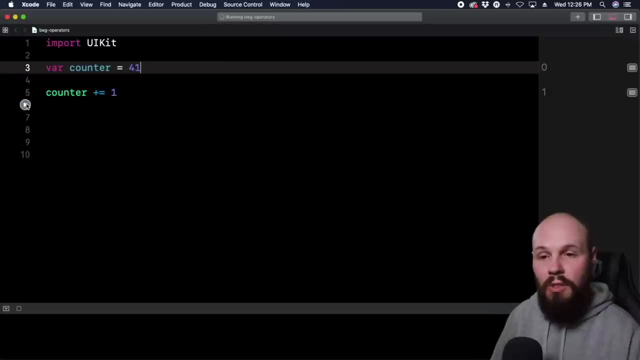 is basically adding one to whatever the current value of the counter is. So let's run it. You see, over here on the right, we get the one And let's say: if this was, you know, 41,, now our counter is going to be 42,, as you can see. So we're just incrementing the number. 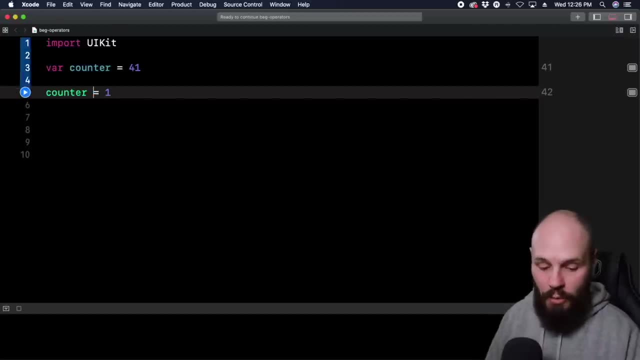 by one. You can also decrement which is subtract by doing minus equals. So if you ever want to like keep a count of something, a counter is very common. If, like every time a user does an action, you want to increase the count, You do, you know whatever. 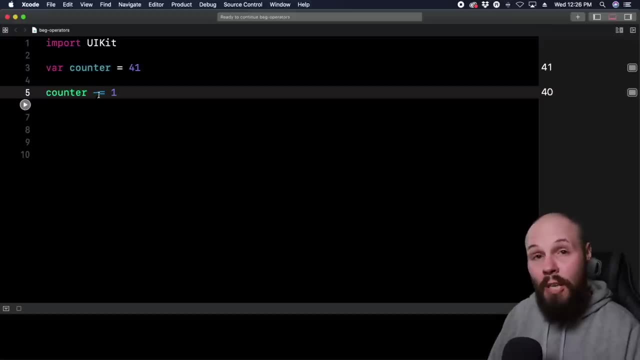 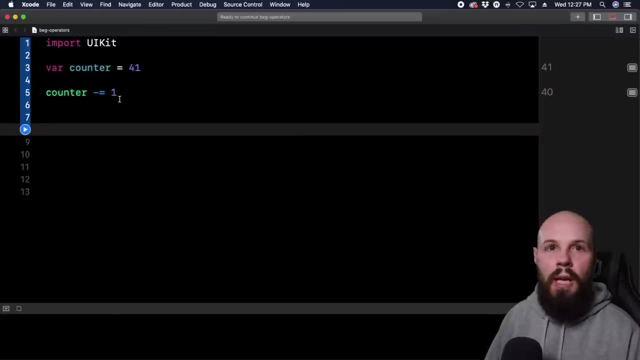 it is plus equals one, that'll increment it by one. And again you can also decrement by minus equals one to lower the count by one. And then, lastly, you can use the plus icon here to add strings and arrays together. So let's say: let greeting equal hello and let name equal Sean. 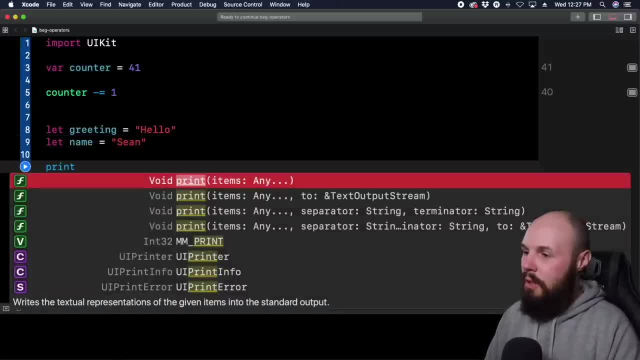 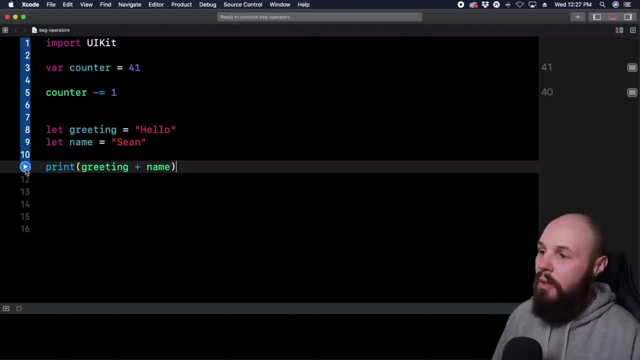 So I can do print And then the message is greeting plus name. So we're adding two strings together And you'll see the greeting that gets printed will be: Hello Sean, I forgot to add a space, Right, So you just put it together a little. 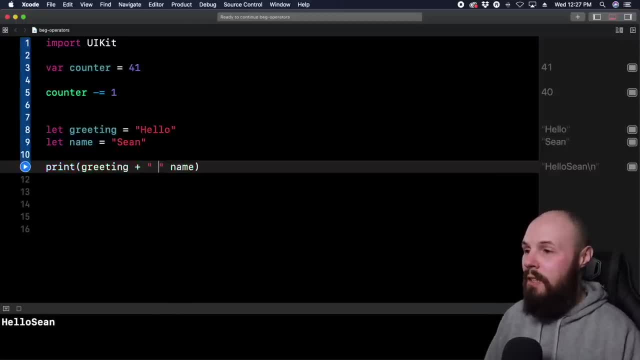 unintentional lesson here. So I can do a space there, That's the space, and then another plus. So you can like really keep adding these together. So now it's going to be the greeting plus space, plus name, And then you'll see, now it's going to equal: Hello, Sean. So again, 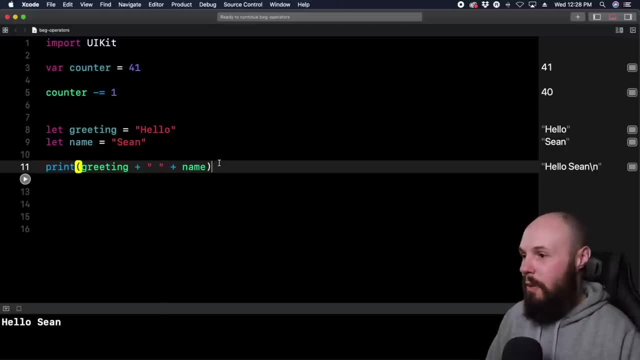 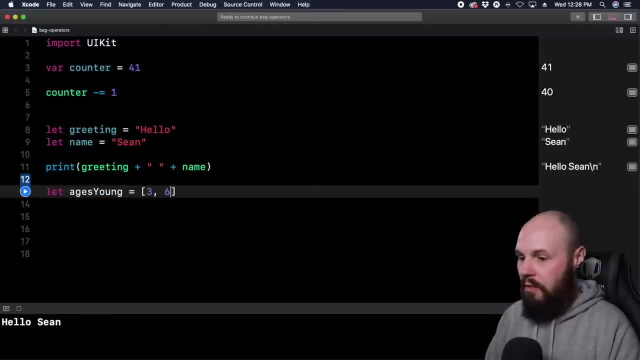 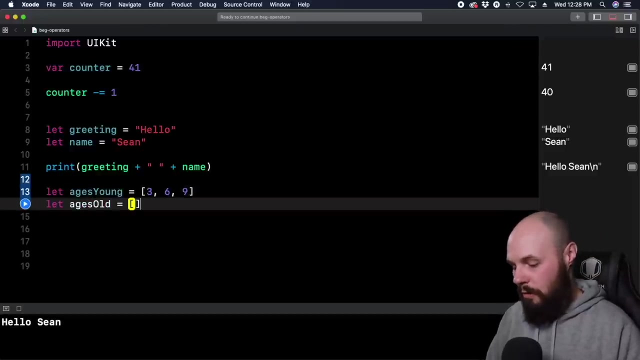 you can add strings together, you can even do it with arrays. Say: we have let ages young equal, you know three, six, nine, someone finish it. And then we do let ages old equal, you know 99, comma, four comma, that's not old- 67,, whatever that's it. And then 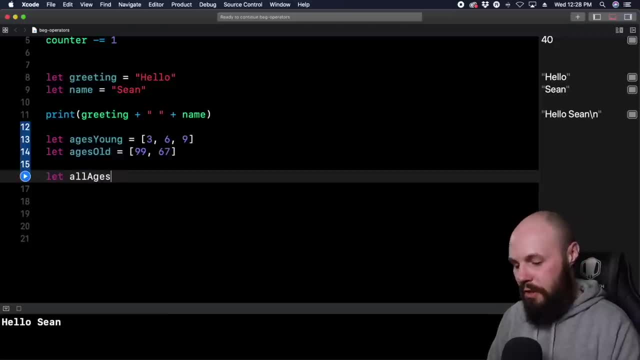 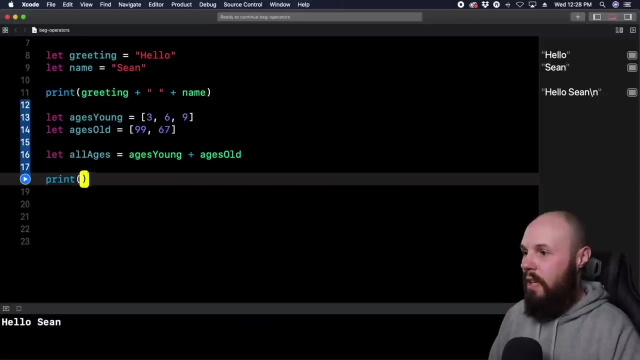 now we can do: let all ages equal, ages young plus ages old, and what's going to happen is ages old will get added on to the end of ages young and it'll be one combined array. So we do print And we want to print all ages. Let's run that. we're going to get the 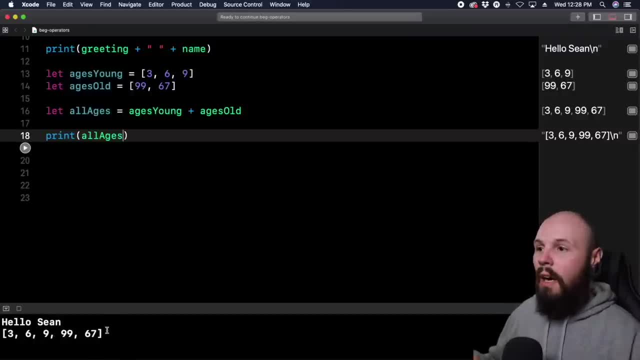 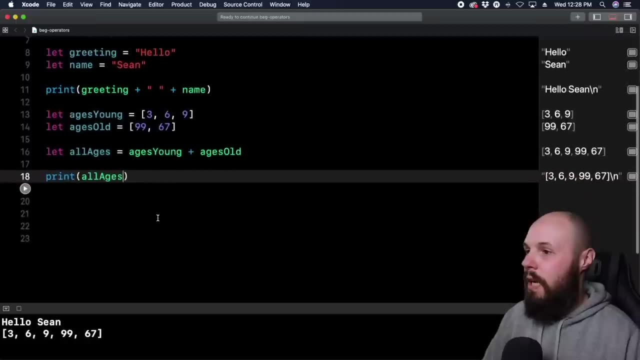 you see three, six, nine, and then 99,, 67. So again, these operators can be used in many different ways. We only scratched the surface here, But again, basics course. So hopefully you understood those basic operators. As always, if you have questions. 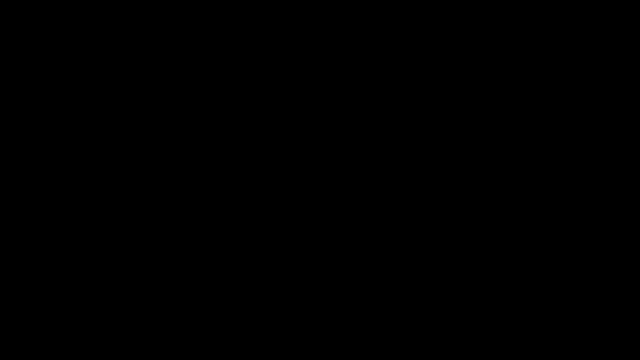 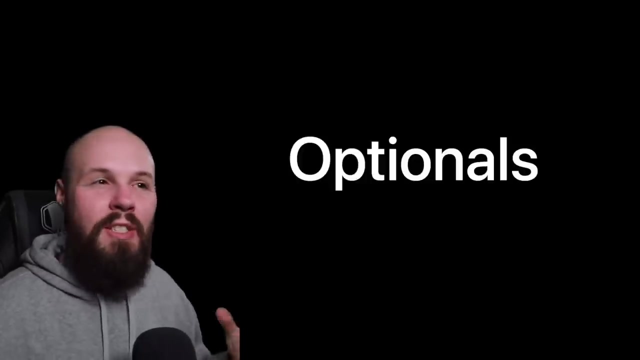 leave in the comments or hit us up in the Slack channel. See you in the next video. All right, we're on to our first tricky topic and a topic that hangs up a lot of beginner developers, And that is optionals: Declaring something as a 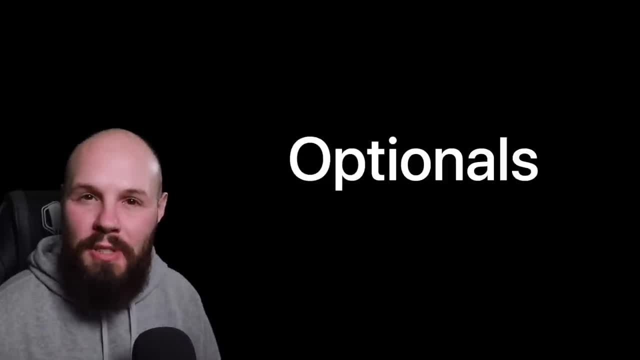 optional means you're giving it the ability to handle the absence of value. Before I give you the basic explanation, let's dive right into this playground to talk about an example that we saw in a previous video. So here in this new playground, you can create your new playground and copy this. 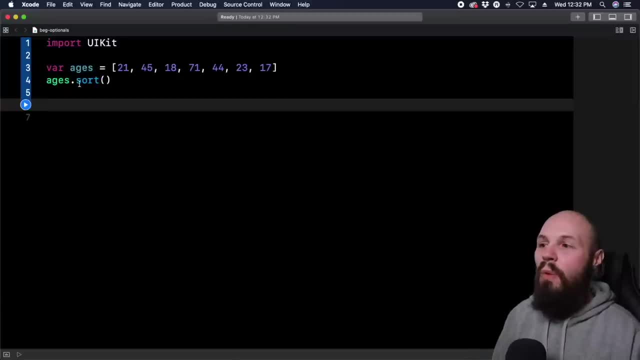 if you like. Remember we had our ages array And let's say we want to get the oldest age of all of our students right, That was all in the array. So let oldest age equal. and remember we did this: ages dot last, Do you remember? 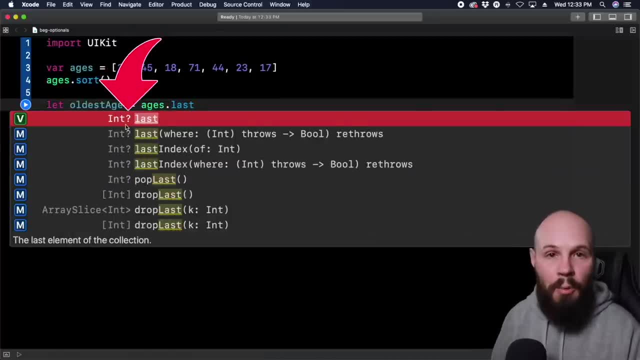 And I said this question mark means ages. dot last is an optional. And the reason it's an optional, remember, because ages could be an empty array And there's no last item in an empty array, right? So that's why it can either be a value, which in our case would be 71,, as that's the 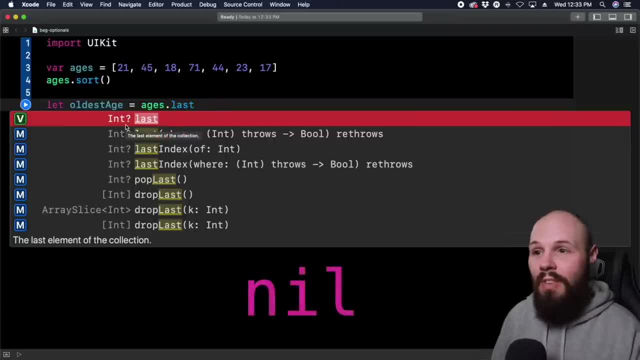 oldest age in there- Or it could be nil, the absence of value, if the array is empty. So that's what the optional does, is it gives you the ability to either handle the value or handle nil. So let me hit return here And let's run it, And you'll see that it's empty And it's empty, And it's. 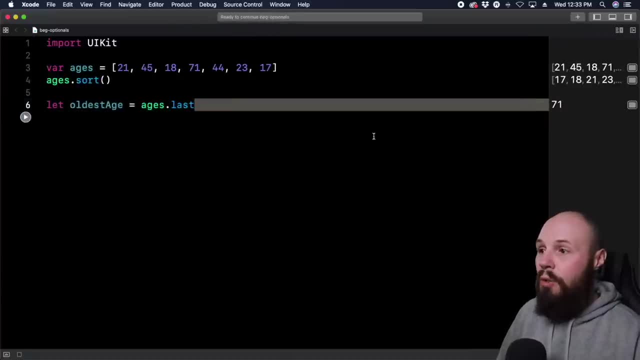 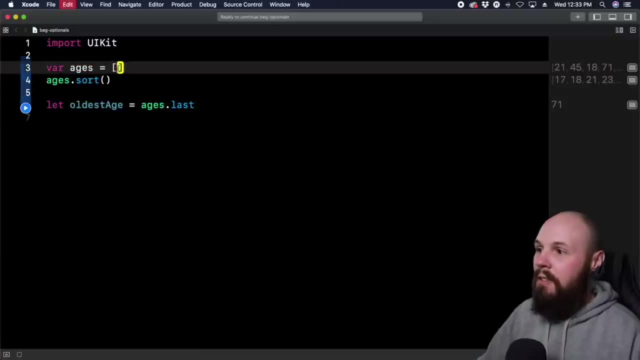 empty. We get the 71 over here. right, That is our oldest age, 71.. Because we sorted the array here, ages dot sort. Now let me give that empty array example. I'll do command x so I don't have to. 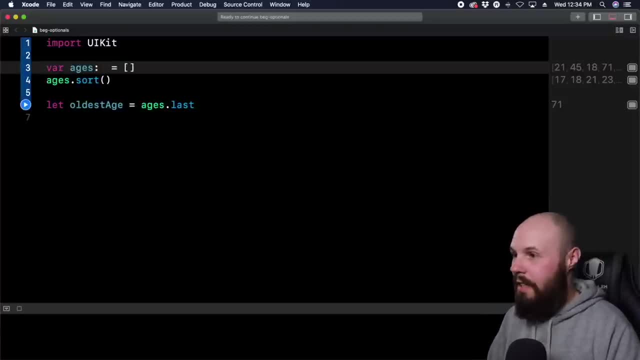 type them again. And then I have to give this a type now because it's an empty array And it needs to know. So we put int in the square brackets. let it know, it's an array of ints. And now when we run, 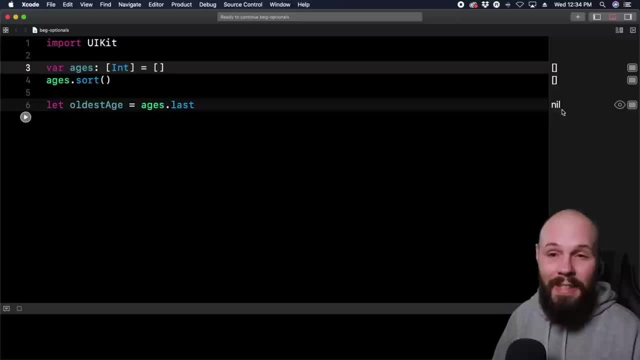 it oldest age is going to be nil, As you can see here on the right, it is nil, And that is the absence of value. So, Swift, giving you that flexibility to handle both, is great. However, what I just said is you as a developer have to handle both cases, So when you write your code, 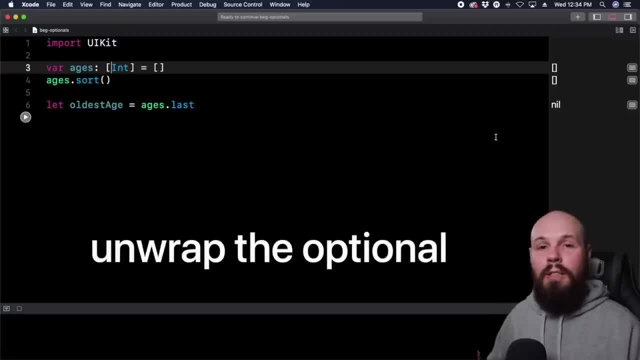 you have to do what we call unwrapping the optional to see if it's either nil or if it's a value. you know, you write the code to handle it when it's a value And then you also write the code to handle it when it's a nil case, And that's what we're going to talk about in this video is. 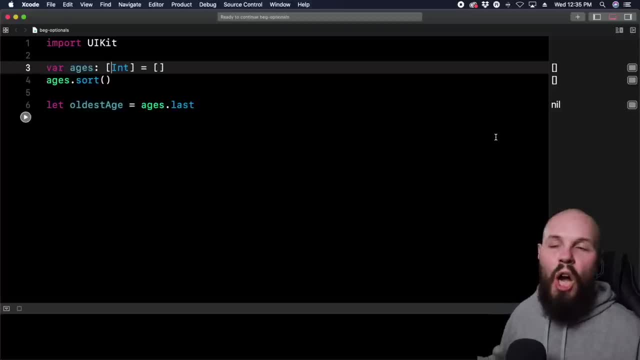 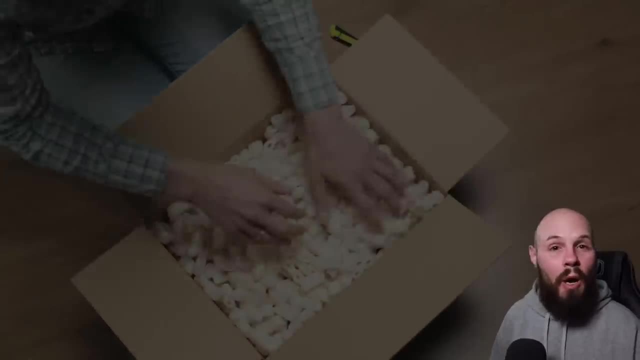 what the optional is and how to unwrap them. So the most common way to describe what an optional is is: imagine an optional is like a box. you don't know what's in that box. It's a closed box. right The box. 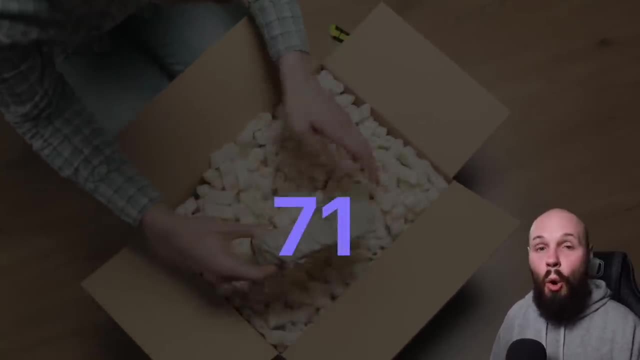 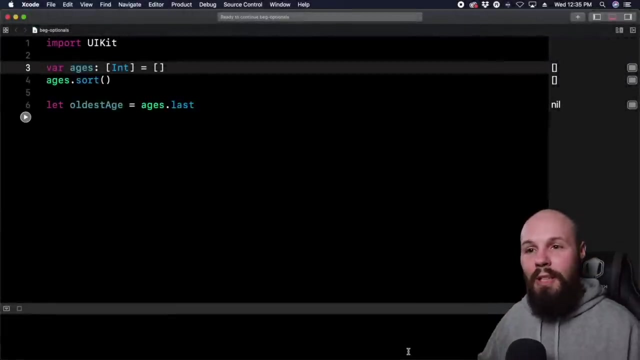 could have the value in it, in this case the number 71, or it could have nil. you don't know what's in the box until you unwrap it. that's unwrapping the optional. Now, the reason you have to unwrap it and handle both cases, like we mentioned, is because if you just use that box, 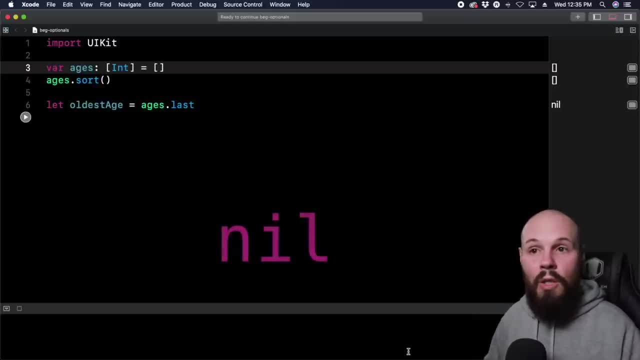 and expect it to have a value, and then it ends up having a nil: your, your apps not going to behave correctly or, in most cases, it'll probably even crash because you didn't handle the nil properly. And remember I said that like, take a second, remember most of your crashes when you're 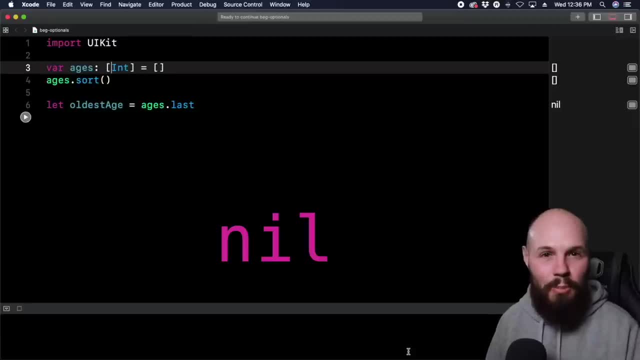 uh, building an app will come from you not handling a nil case properly, right You're. you'll run a program. it'll expect a value. that value will be nil and your app will crash. You're going to see that a thousand times throughout your career. Very common, So again in this video. 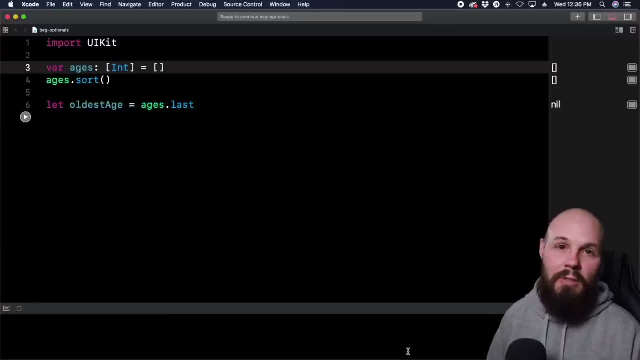 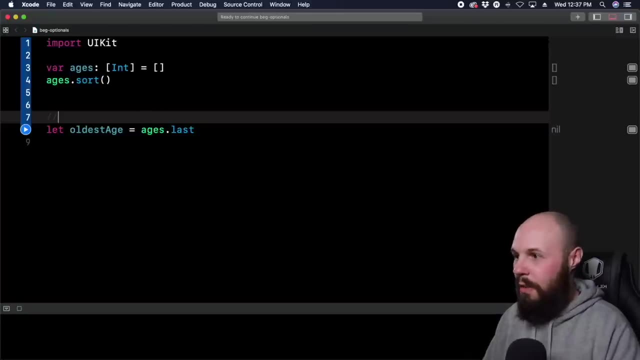 we're going to talk about how to properly unwrap and handle the nil cases. So let's work with this oldest age variable and unwrap it. So the first way: there's actually four ways we're going to do this. This- we'll comment this if let is one way: nil- I'm going to spell this wrong for sure. coalescing. 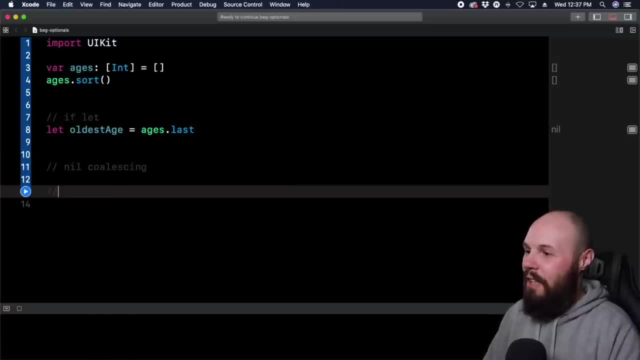 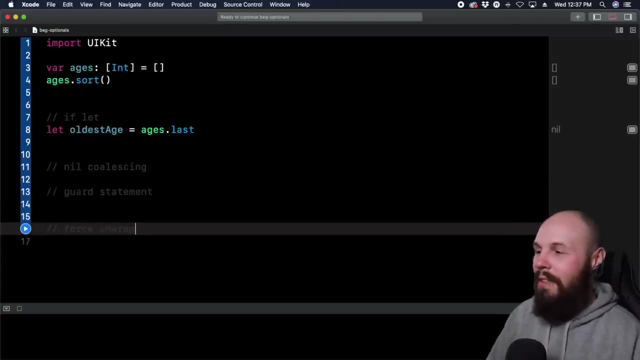 I for sure spelled that wrong, probably. And then there's the guard statement, And then there's the dangerous. we'll explain why force unwrap. we'll get back to that in a second, But I want to. I wanted to list those out real quick And I'll leave the comments in the playground, Hopefully. 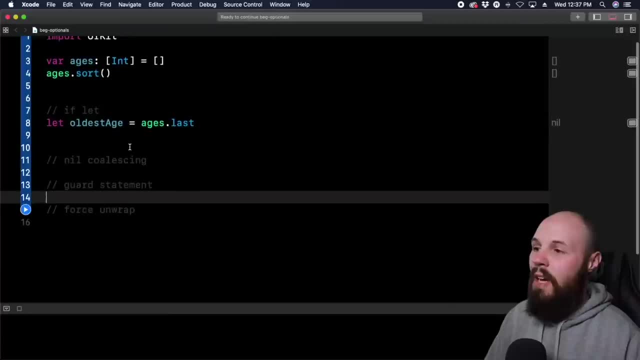 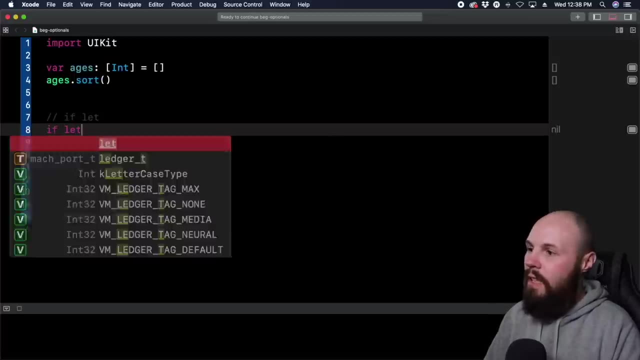 you put them in the playground as well, So you can have the names of how to do this. So the first one is: if let- I'm actually going to delete that so we can write it from scratch. So you do. if let. oldest age- and we're giving it the name here- equals 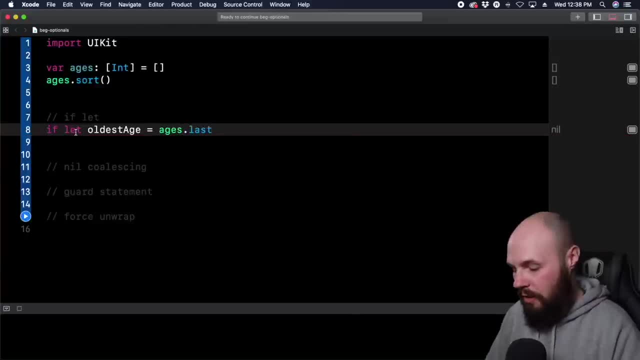 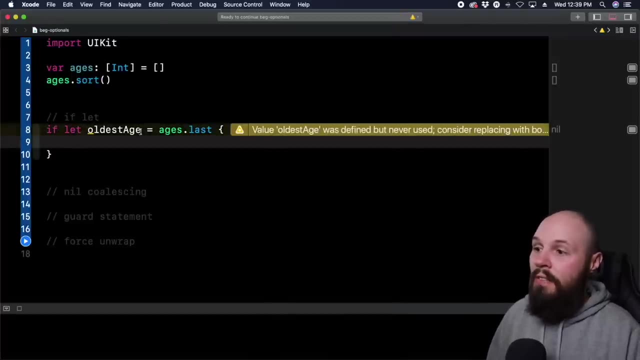 ages dot last And this is the optional. So here's how this read. Well, actually, let me give it the open and close curly brace, because we have to set the scope of our if let statement. So we're saying is if ages dot last has a value, right, if it's not nil. if we open up that box and it actually 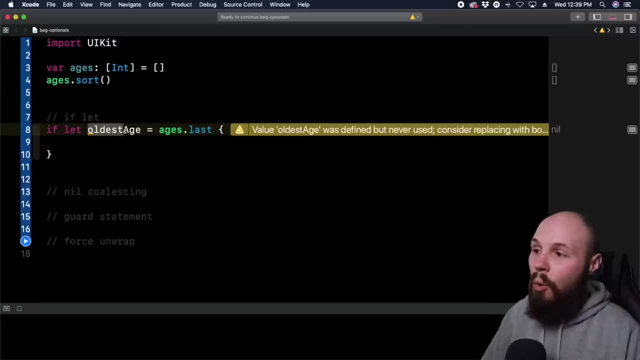 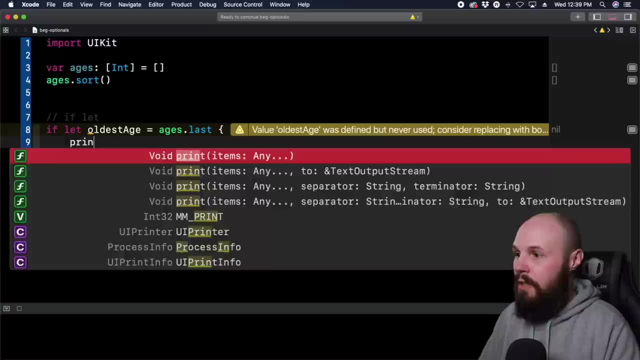 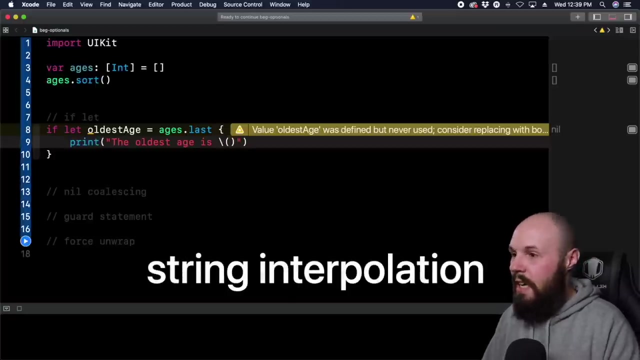 has the value in it. then give that value a name: oldest aged. we're storing it in a variable And now we have access to that variable within this scope. So now we would do print the oldest age is what's called string interpolation. you do the forward slash and then the parentheses, And then 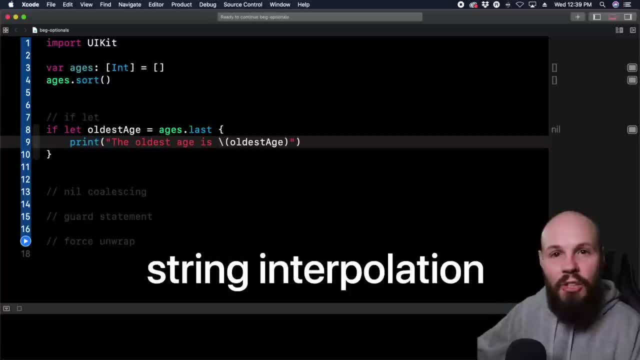 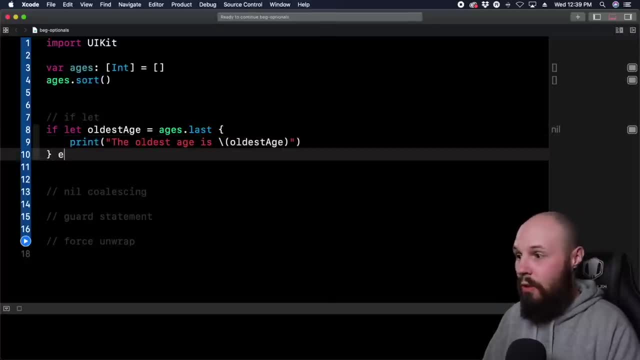 here you can pass in the variable oldest age, because that's an int, right? An int is not a string. So in order to put something into a string like an int, you have to use string interpolation, And then now we do the L statement, for if it's nil, Now we want to do print. there is no oldest. 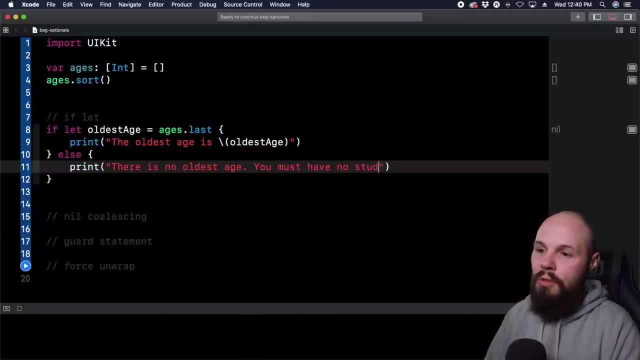 age, you must have no students, meaning the array is empty. So again, right now, the array is empty. Let me, let me run through this again before I run it. So what we're saying here is: if ages dot last has a value, right then assign it to this variable called oldest age. And now we 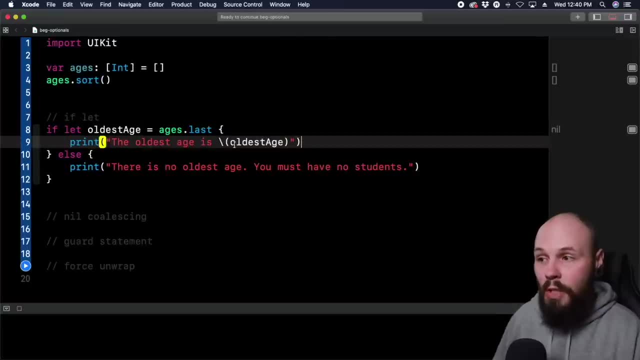 can only use oldest age within this scope right here, And that's where we're using it to say the oldest age is blank. And then the L statement fires off if it's nil. So if it's nil, meaning there's no value, you would say there is no oldest age, you must have no students. And in real life, 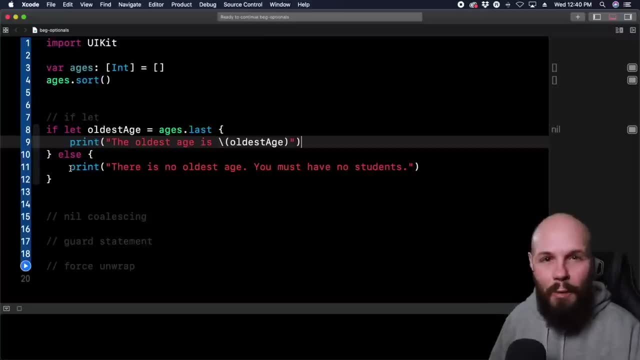 when something's no. this is where you'll probably pop up like an error message or something. But you know you don't always have to just do print statements. So right now the array is empty, Let's run it, And we should go into our nil case, right? Yep, there is no oldest age. 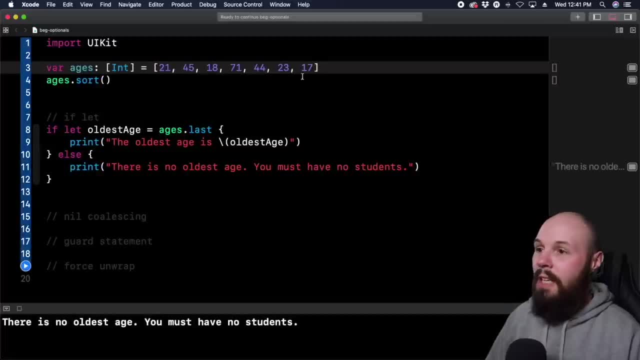 you must have no students. Let me do a command V here to paste back in our ages. And now let's run it, Because now we do ages, dot last is going to have a value: it's going to be 71. Now let's. 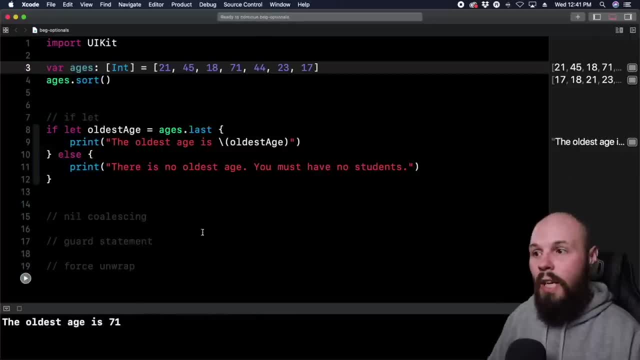 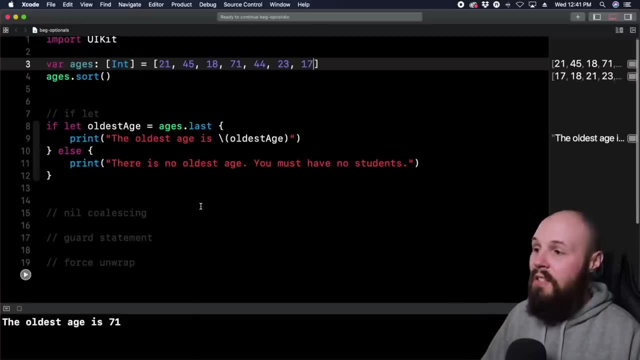 run it And the oldest age is 71. So again, we unwrap the optional. depending on what's in the box, a value or no, we handle both cases properly. So that's the if let statement. that's kind of a. 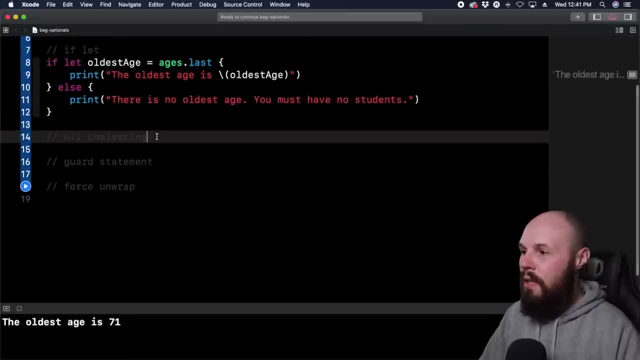 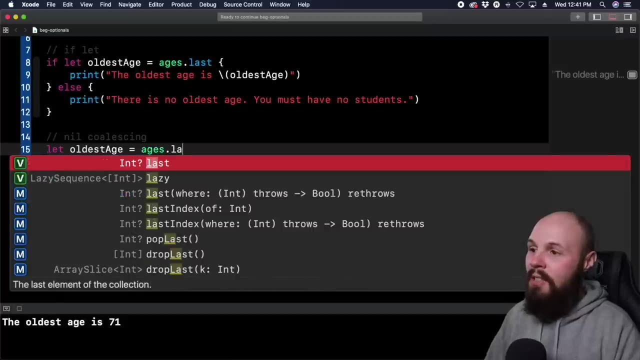 little bit verbose. No, coalescing is a little bit simpler. So here we can do: let oldest age equal ages dot last. And here is where we can give it a default value. So we're, we can do question mark, question mark, and then now we have to give it an int. 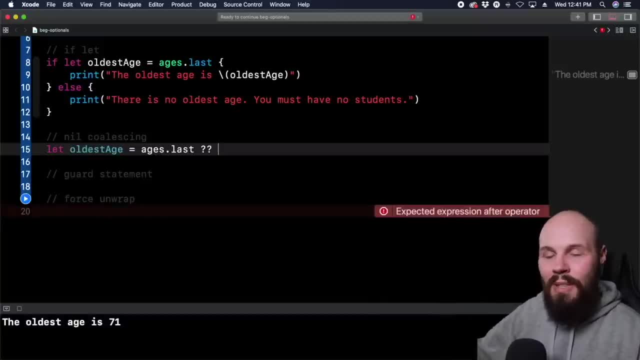 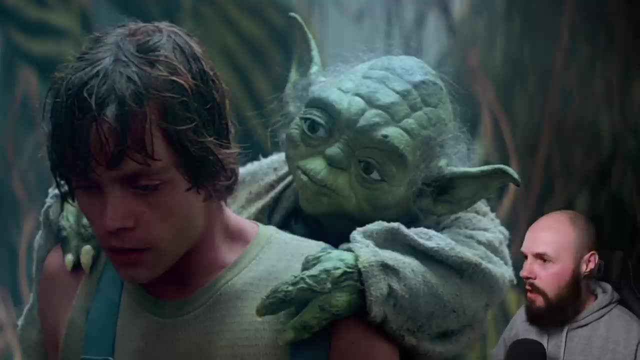 So here's where, in this case, it might not be useful, because I have to give it an age. So let's say: you know, I want to do 999, which is obviously not a real age. I think that's your Yoda. So what is what this is saying here is: okay, let's create this variable oldest age if 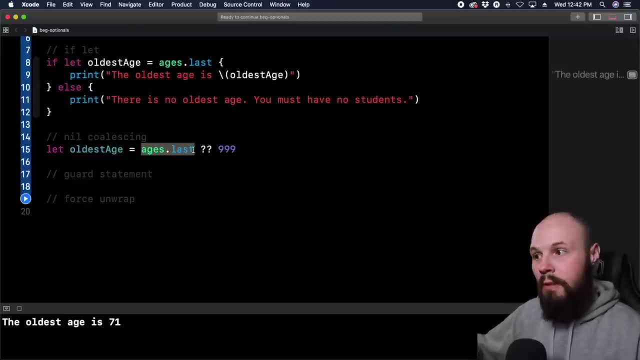 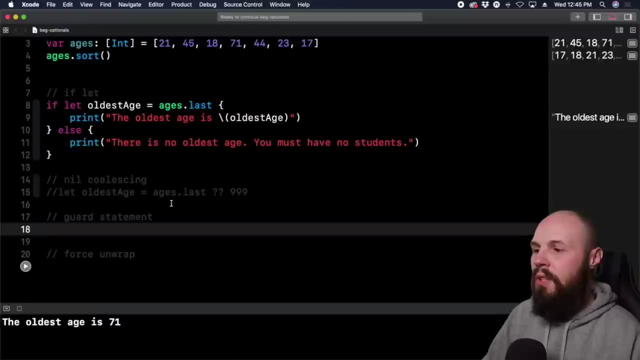 that last has a value, right, we unwrap the optional. if there's a value in there, cool, That's what oldest ages. if there's nil, we give it a default value of, in this case, 999.. Now to use a guard statement, we have to be in a function because a guard statement has. 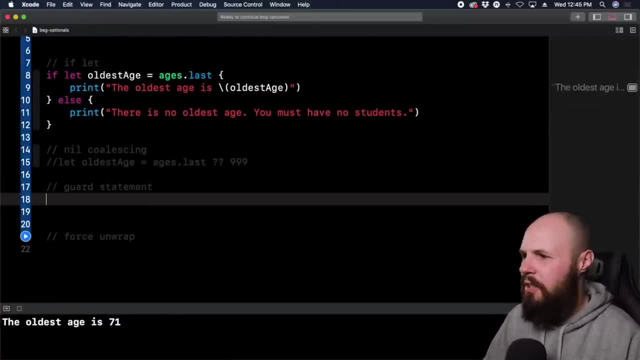 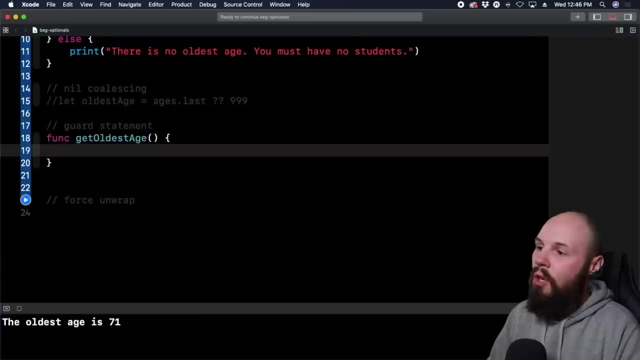 to return has to have an early exit. that will make sense when I actually show it to you. So let's write a quick function funk. get oldest age right And here we can do guard. let oldest age equal ages. dot last looking, looking very familiar so far. 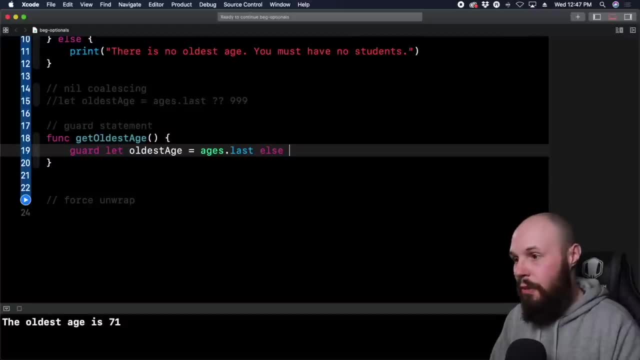 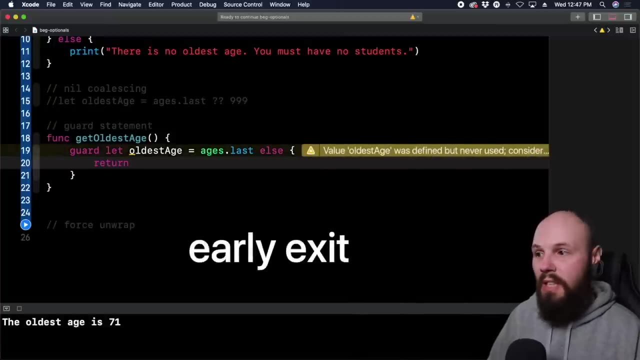 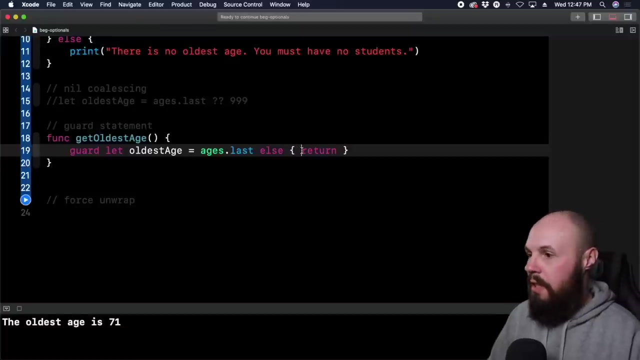 and here's where it differs else. and then you have to return if it's nil. so what guard does is it gives you what's called an early exit if it is nil, and oftentimes you may see this on one line like that. just to avoid confusion I'll put it on the second line, just so you know. 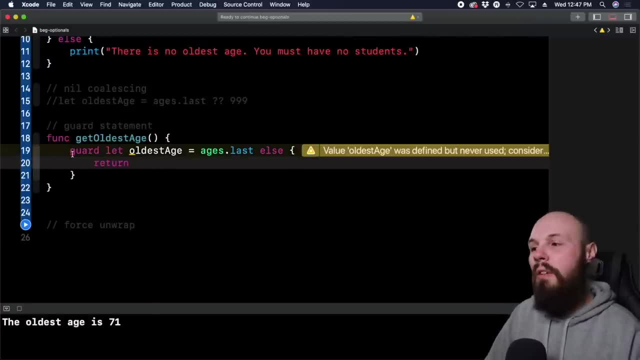 that that's what's happening, because when I explain it here- and a big benefit of using a guard statement is oftentimes it can clean up code- I like to call it like a line in the sand, like you're drawing a line here, because what happens is nothing will get executed after the. 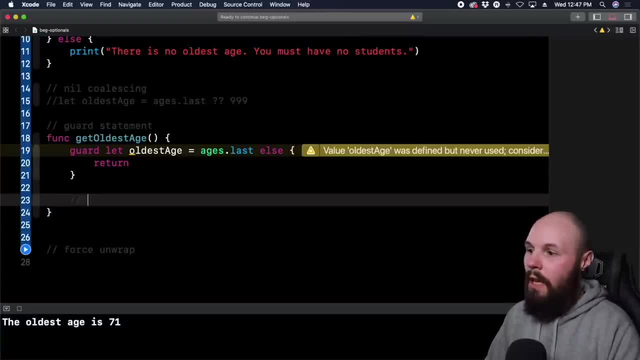 guard statement. like, let's say you had a bunch of- uh, you know a lot of code down here in this function. well, basically what the guard statement does is: you know if ages dot last uh has a value, go ahead and assign it the oldest age and if, if not, return like, stop the function. that's why I 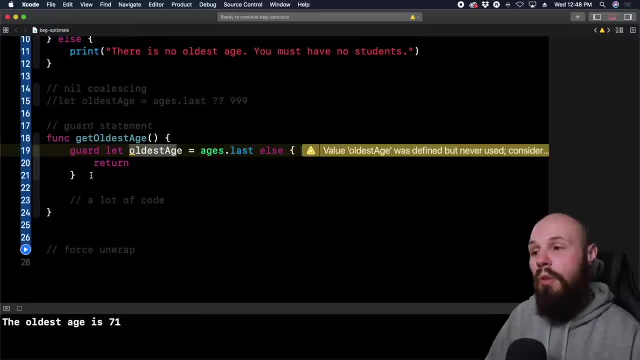 call it a line in the sand. nothing happens below, like nothing will happen below this return. if oldest age is nil, because oftentimes when you're writing functions like if the value you're trying to get is nil, then you're going to have a line in the sand and you're going to have a line in the 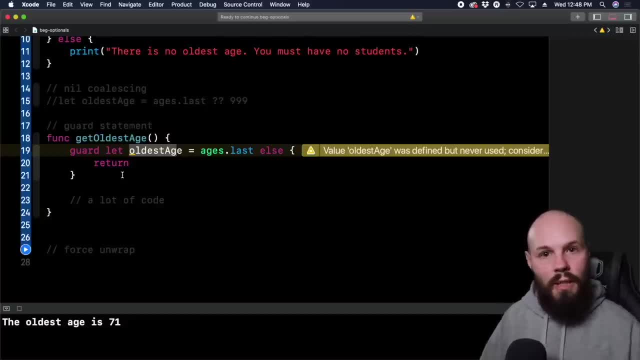 sand and you're going to use a lot is nil, like you don't want to execute all that code because you need that value. so again, this gives you an early exit out of the function. should you get nil and then oftentimes in this return block here, this is where you would show like an error alert. 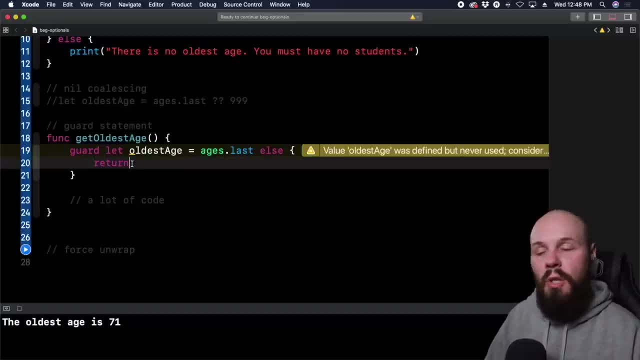 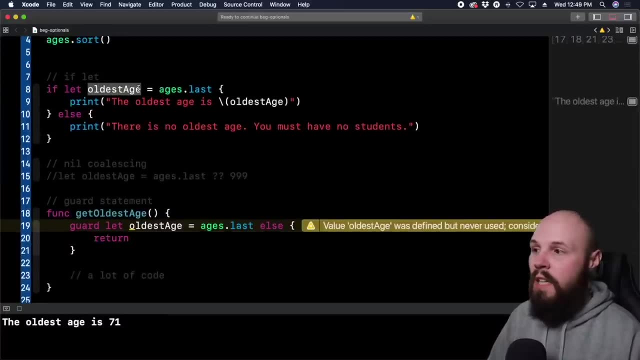 saying: hey, we didn't get the value. sorry, um, but for now we're just returning, getting out of the function. but the difference between if let and guard let is remember if let gave you access to this oldest age variable only within this scope, right here. so you could imagine if you're checking. 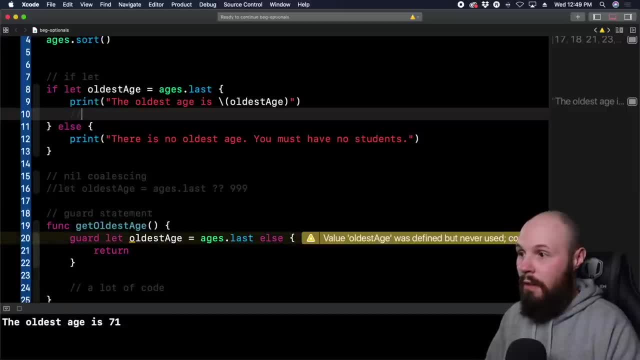 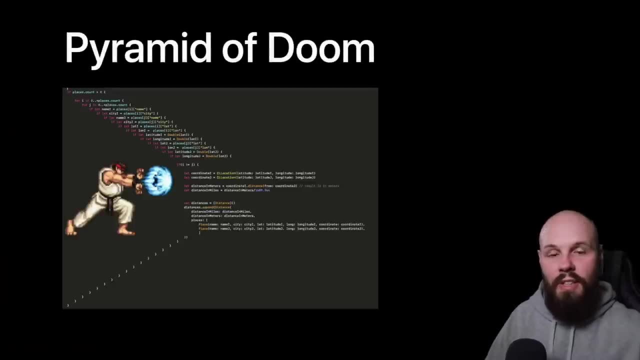 for the option in the beginning. now you have, you know, a lot of code down here. uh, it can get real. it's called the pyramid of doom, where you have like if, let, if, if, if, and it just becomes a giant like pyramid of code. um, so guard, avoids that again by 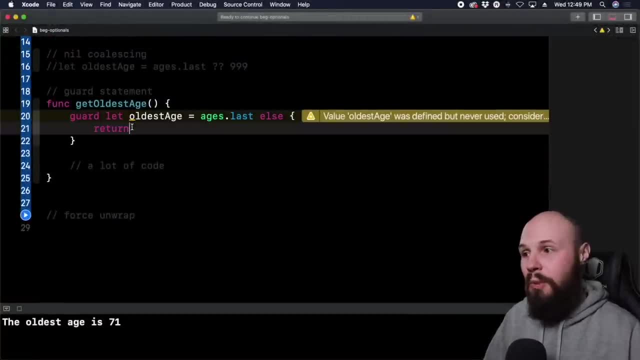 checking for the value up front, and if it doesn't have it, you get out. if it does have it now you have access to oldest age in the entire scope of the function, not just the scope. uh, like, have if let was just its own, its own scope. you have it in the entire scope of the function. now we'll do. 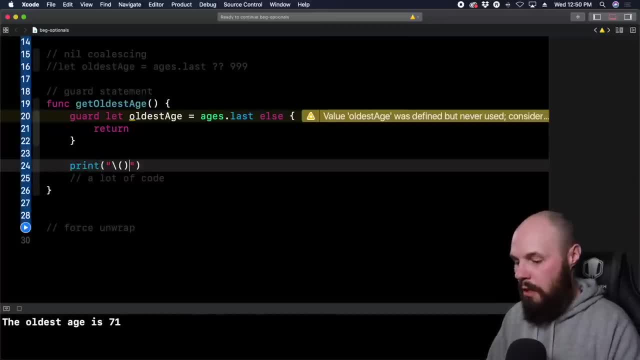 some string and we'll do some string interpolation again. uh, oldest age is the oldest uh age, so 71 is the oldest age. but, like i said, i have access to this oldest age variable just in the scope of my function. it doesn't go into the pyramid. so, uh, guard is nice one for the early exit and it cleans. 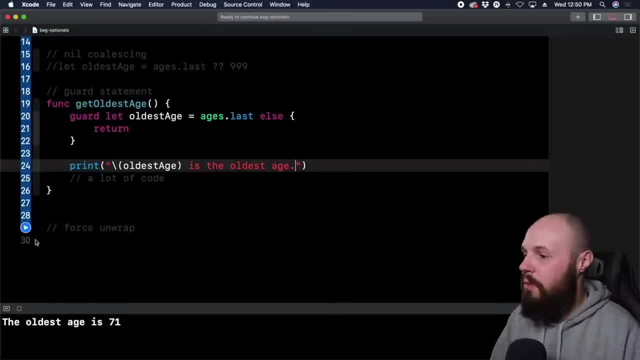 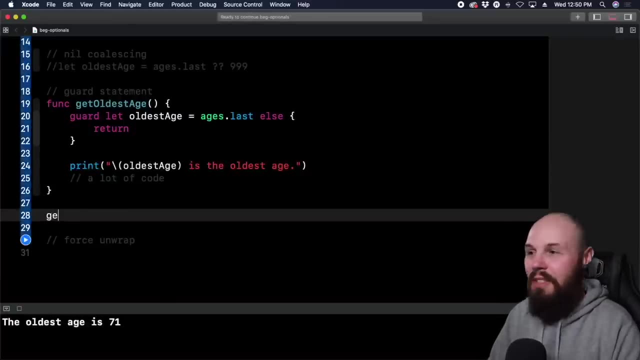 up. your code avoids what we call the pyramid of doom. uh, so now let's run this real quick and you'll see it now prints off. uh, yep, i forgot to call the function. as always, always happens. it's happened to you a ton of time to uh, get oldest age right there. so now that we execute, get oldest. 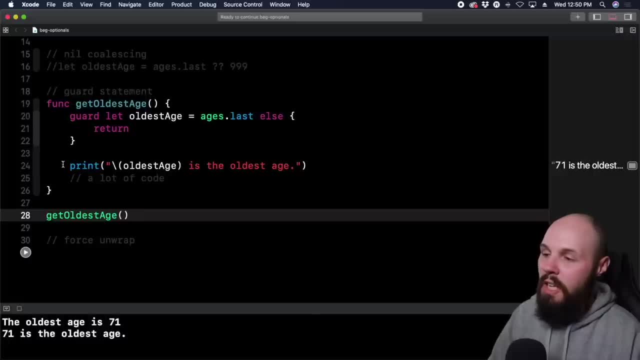 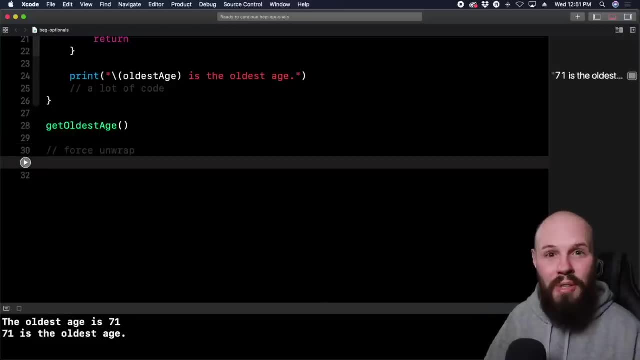 age. uh, now we print: 71 is the oldest age. that's this print statement right here. so now, finally, the force unwrap. this is the. this is super dangerous because it's like the, the cheat code, the easy way out. uh, so you would just do: let oldest uh age, equal uh ages dot last and just put. 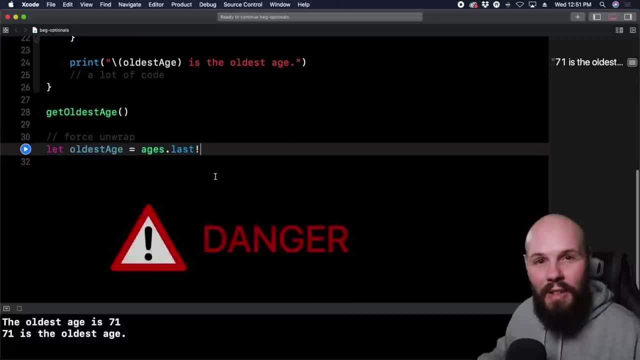 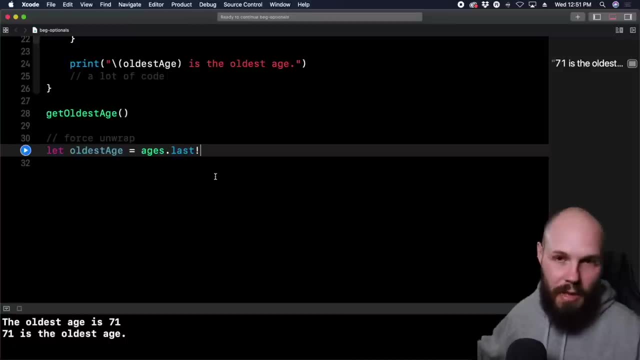 an exclamation point on there to the bang and basically what this is saying. this is why this is going on. some developers will say: never force unwrap an optional in any of the code bases. right, i'm of the opinion that sometimes it makes sense, but definitely by far like the rule of thumb is to 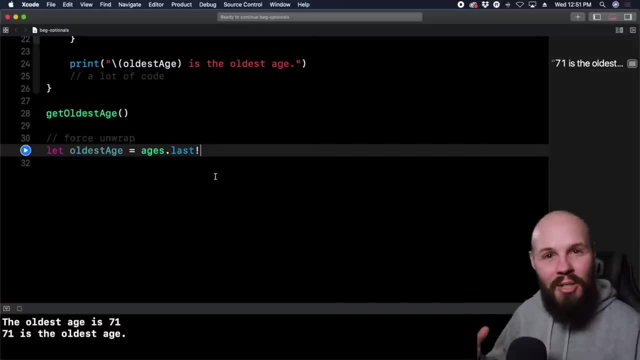 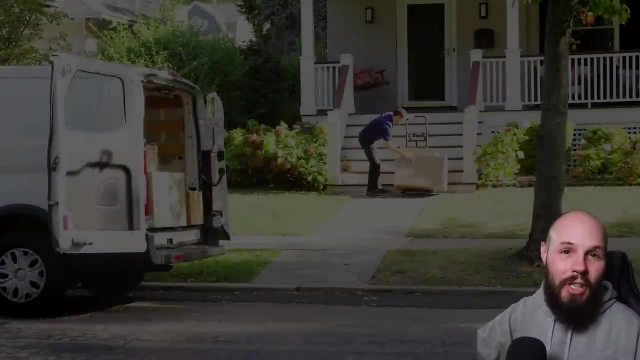 not use force unwrapping, because what that does is remember that box that either has the value or a nil. you're basically saying: i don't care what's in this box, use it, and this is where your crashes are going to come guaranteed. because you're going to say: don't even look in the box, i don't care. 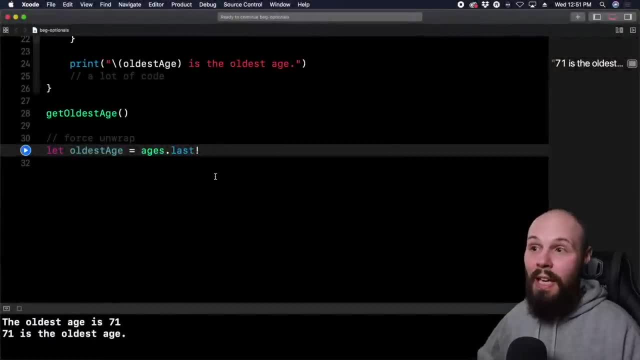 just use it, and then it's going to try to use it and it's going to be nil and crash like this line right here. this, this force, unwrapping, trust me, uh, you will see hundreds thousands of errors, uh, in your code based on trying to do this and again, because what happens? 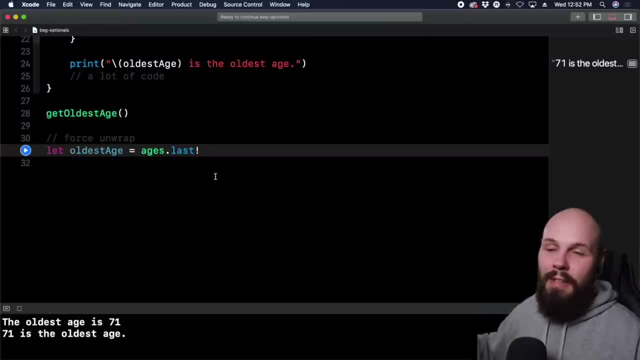 is. you say: use the box, i don't care what's in it, nil is in it- and then crash, crash, crash, crash, crash. so, uh, but that is a way to unwrap optionals and you will see it used like it's not going to be that uncommon. uh, but just know that there's danger when doing it. so that's some basic ways to handle. 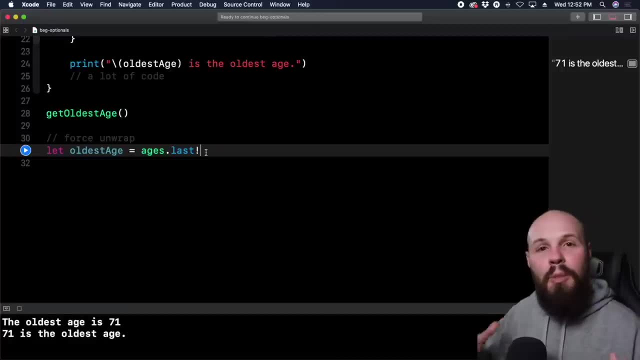 an optional and again, just to really drive the point home, and optional and swift are going to give you the ability to handle the absence of value, which again is like that box: it can either have the value in it or it can be nil, and you have to handle both cases gracefully, or if you force. 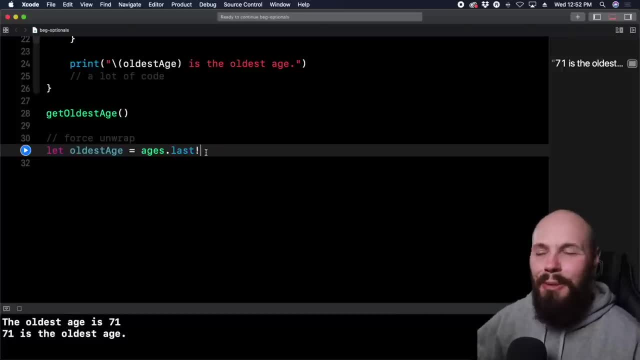 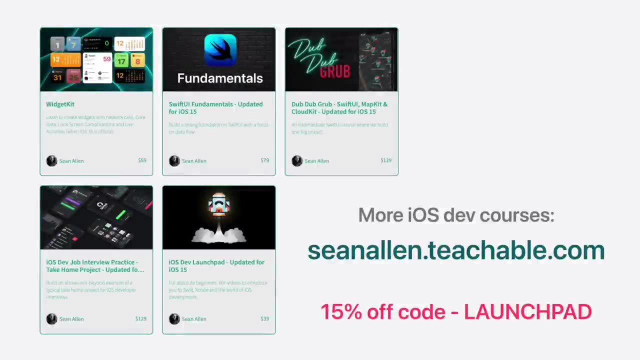 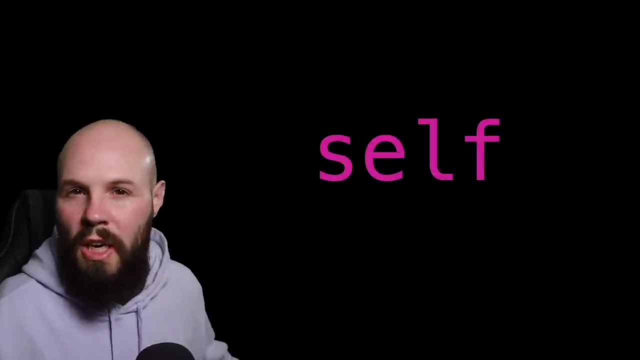 unwrap, you say i don't care, just use it, and uh, that'll, that'll lead to some trouble. but anyway, as always, questions in the comments or in the slack check in the next video. in this video i want to introduce you to the concept of self: self. 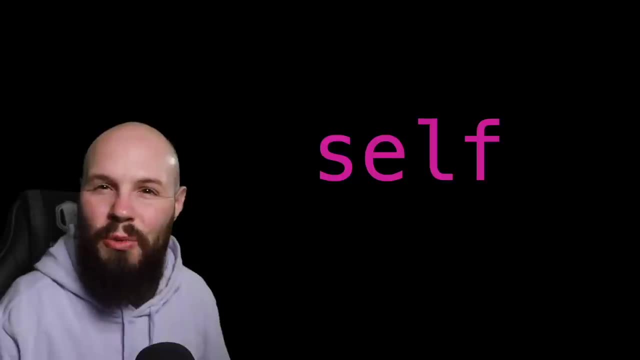 be honest, maybe getting a little ahead of ourselves right now, but we're going to be using this throughout the rest of the course, so i wanted to at least introduce this to you, uh, and then we'll have time to reinforce it as it comes up later on in the course, and the concept of self is actually pretty. 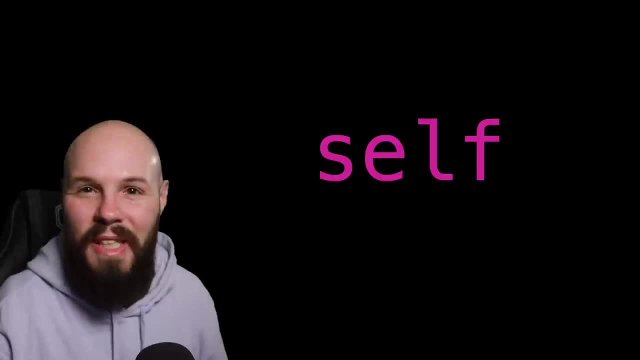 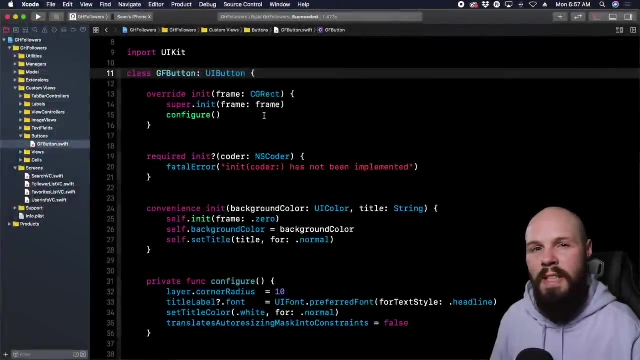 simple. but i remember when i was just learning like i didn't fully understand it because i never took the time to stop and like learn what it was. so that's what we're going to do now. the first example of self is going to be in the initializer for our custom button here, gf button. we're going 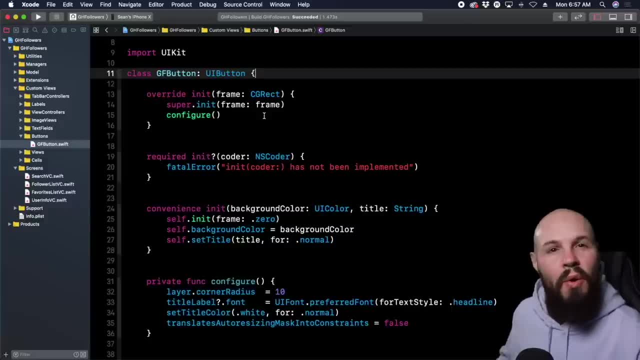 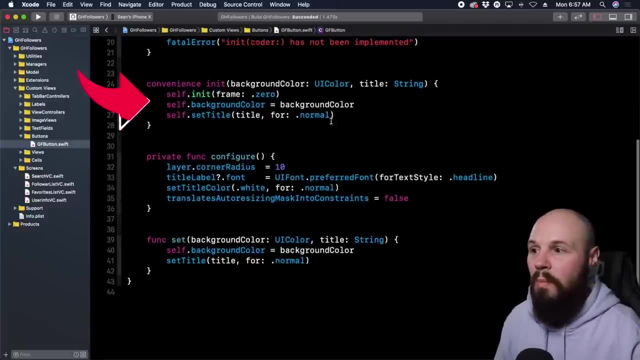 to get into classes and subclasses in the next couple of minutes and then we're going to get into a couple of videos, but let's just focus on the self aspect of this here. so here in the init you can see selfinit, selfbackgroundcolor, selftitle. what self refers to is exactly what it says it's. 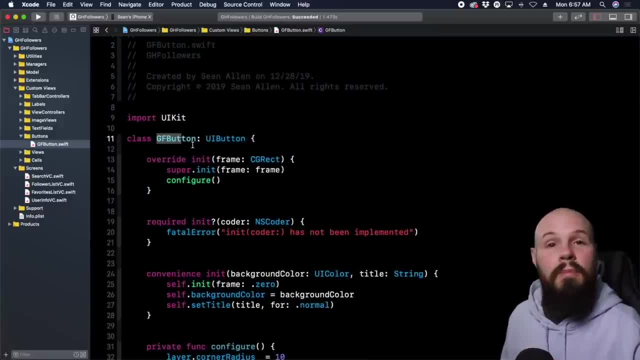 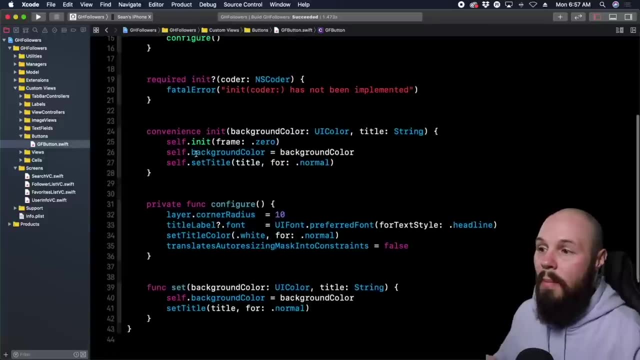 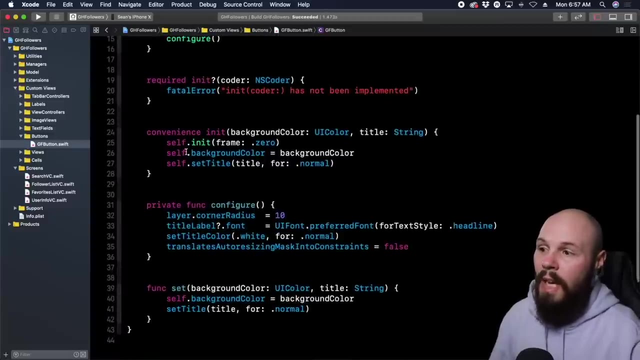 self. so self here is basically the gf button, this current instance of the gf button. so the reason we have to use self in this initializer is because we're saying, hey, make the selfbackgroundcolor means the background color of our gf button equal to background color. and we had to put self here because it doesn't know, like, here's the background color we're. 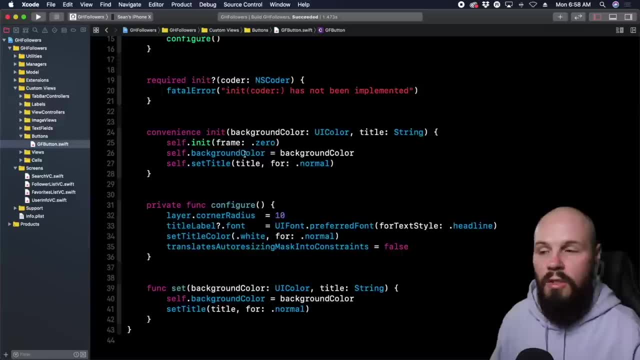 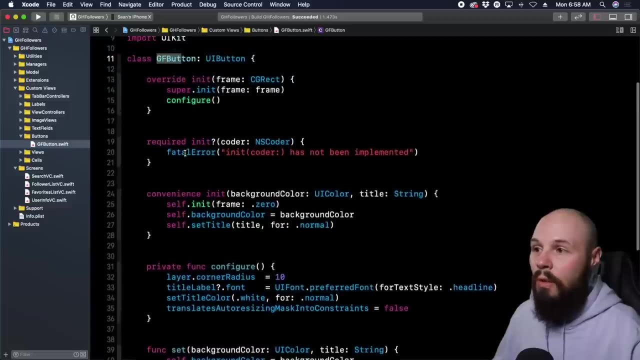 passing in as a parameter what's the same name as this background color. so we need to say hey, set self's background color equal to the background color that we passed in. and again, self refers to the instance of the gf button. let's do another example here: in the favorites list, vc, which again 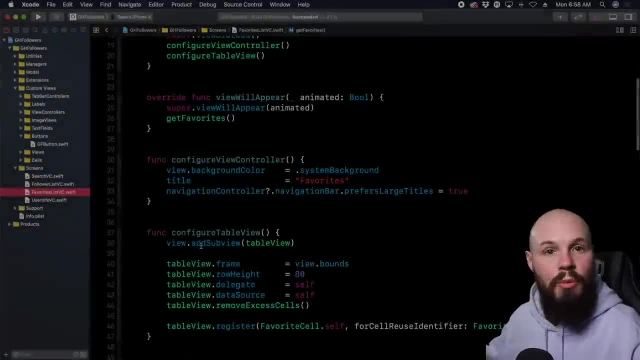 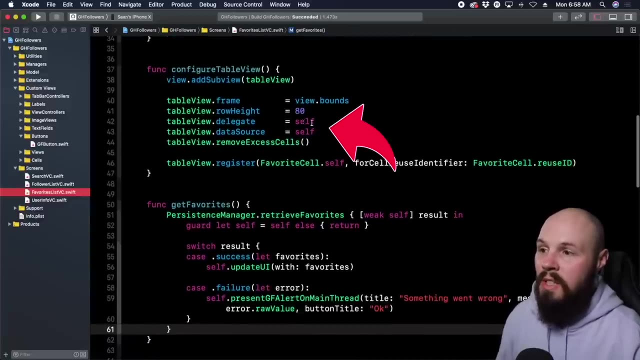 up on the screen is just that table view. well, when you create a table view- which again we'll do later in the course- you have to set delegates, a delegate and a data source. so you can see: tableviewdelegate equals self, tableviewdatasource equals self, and again, self refers to what class. 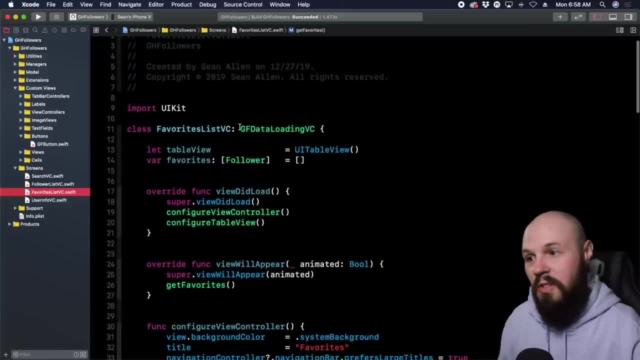 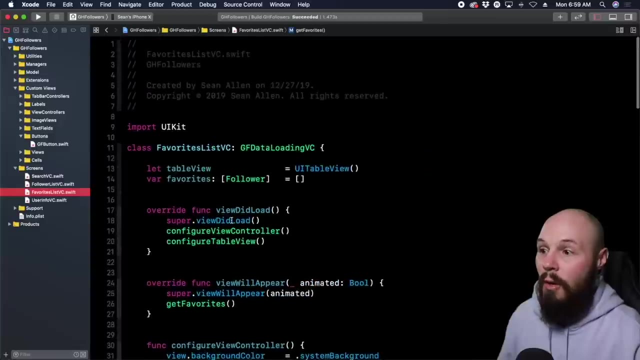 we're in. we're in our favorites list: vc, which is a subclass of gf data loading. vc, which is actually a subclass of ui view controller. again, more on classes and inheritance in the future video. we're focusing on self right now, so again, basically this saying: tableviewdelegate equals our instance. 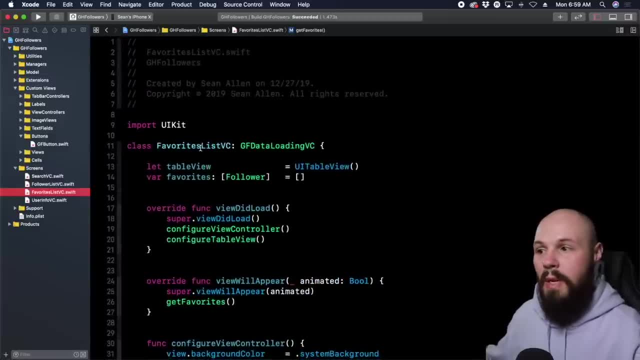 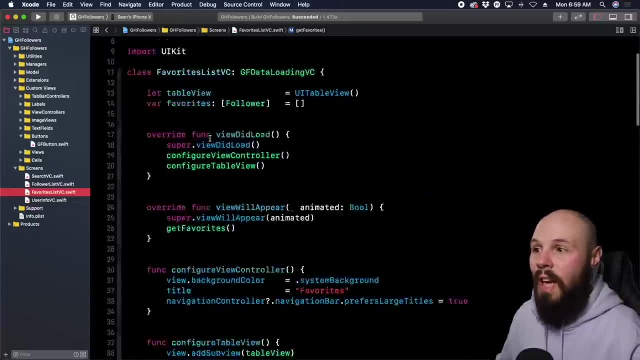 of favorites list vc, which is the screen that shows the table view, that basically connects tableview to the view controller. so that's what self means. self is, again, whatever instance of the class you're in favorites list vc. so again, just an introduction to the concept because, like i said, 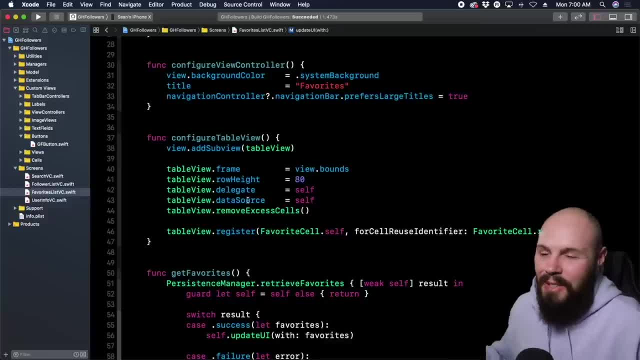 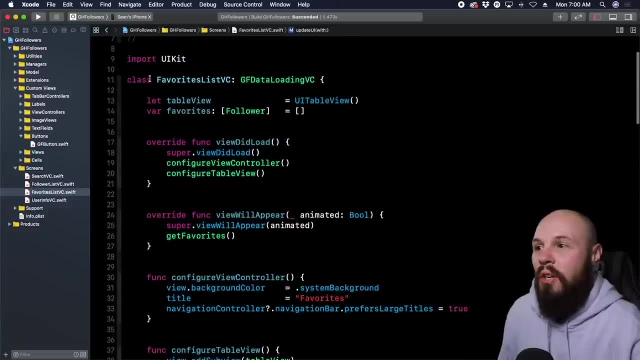 i never fully understood what self meant when i was first starting out, and it's it's so simple when you think about it again. just to drive the point home, self is just kind of a shorthand way of saying this current instance of the, the object or the class that i'm in. so in this case it's the. 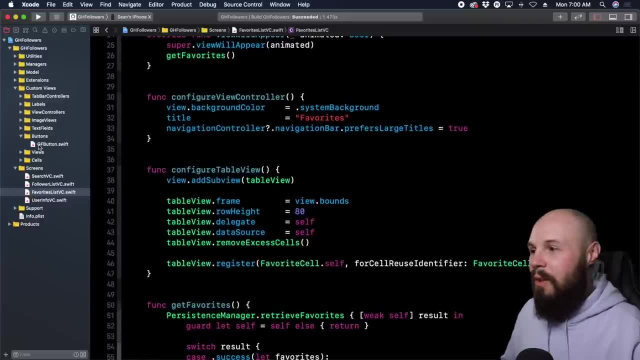 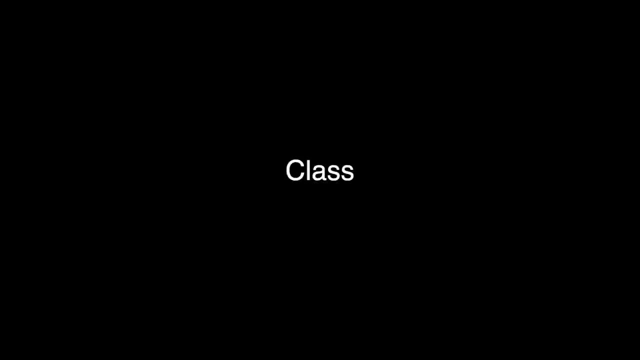 favorites list. vc is what self is equal to all right, so you got a little tease of like subclasses and subclasses. let's go ahead and talk about that in the next video. so let's talk about those classes. a class at a high level is an object. it's one of the building. 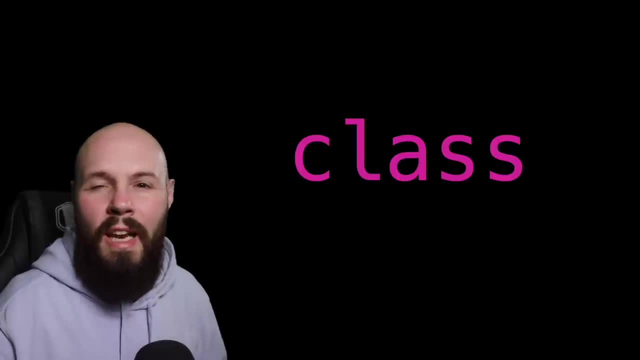 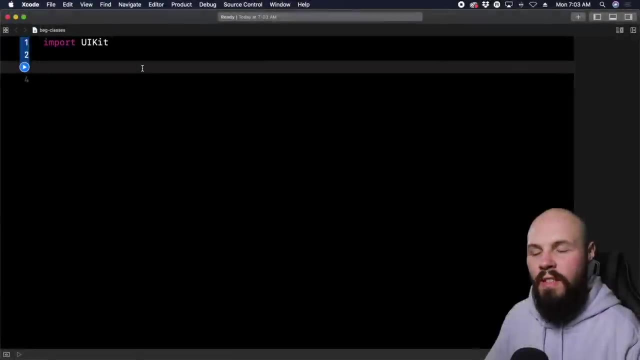 blocks of object-oriented programming and it's an object that can have properties and functions attached to it. let's actually build one. to show you what i'm talking about. we're going to use a version of that developer example we had before. so to declare a class, you type class and then 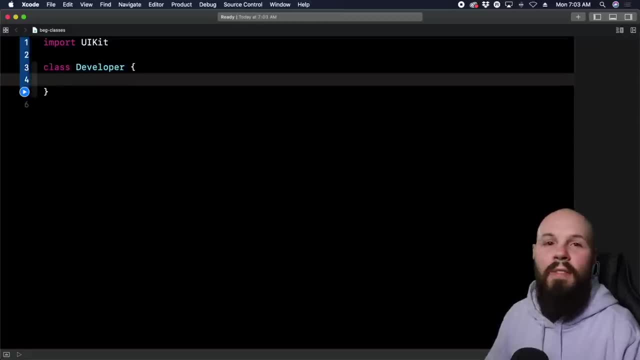 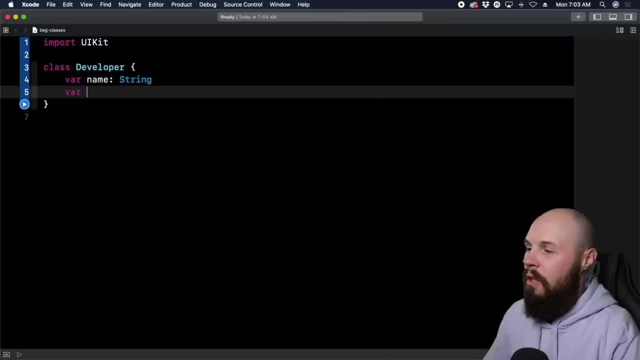 let's call it developer and we're going to call it class, and we're going to call it class and we're going to call it class, and now we need to give it properties. remember, the developer had var name, which is of type string. it had var job title, which was another string, and let's say var years. 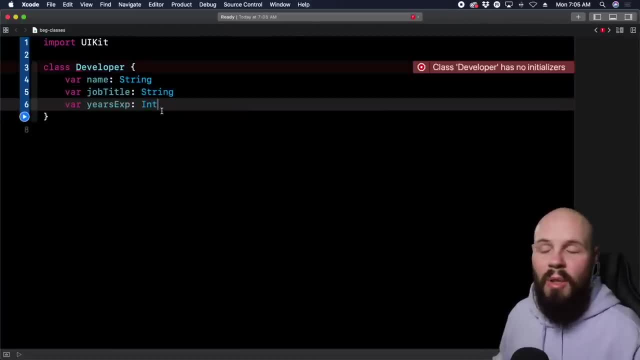 experience, which was going to be an int. so our developer class has these properties: right name, job title, years of experience. now you can see xcode is yelling at me. class developer has no initializers, so when you build a class, you have to tell xcode how to initialize your class and 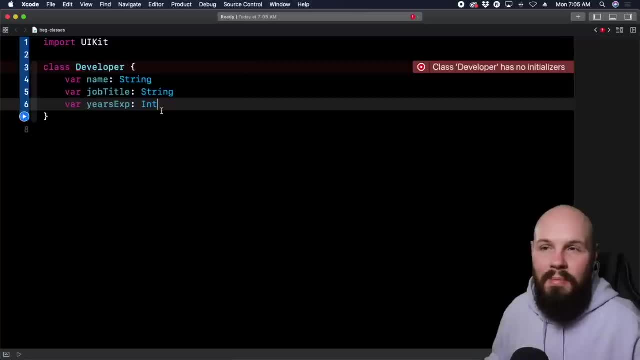 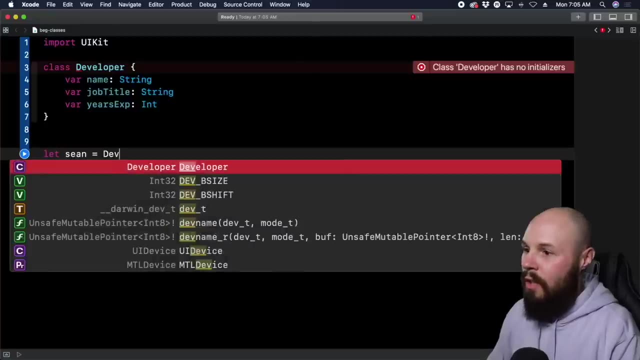 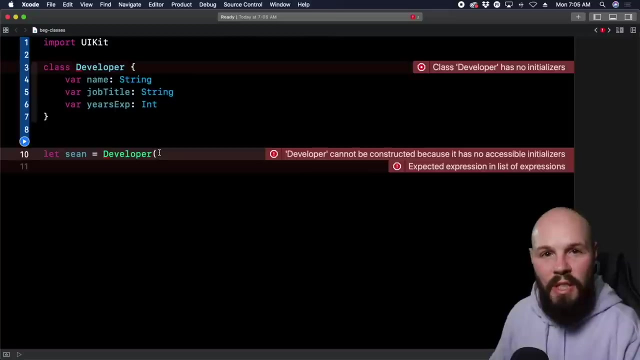 initialize that class. uh, initializing a class basically means creating a new one, so we would want to do something like this: right, let sean equal developer. and remember before we were using, like some initializers, that you saw, uh, in that other developer example. well, we don't have those. 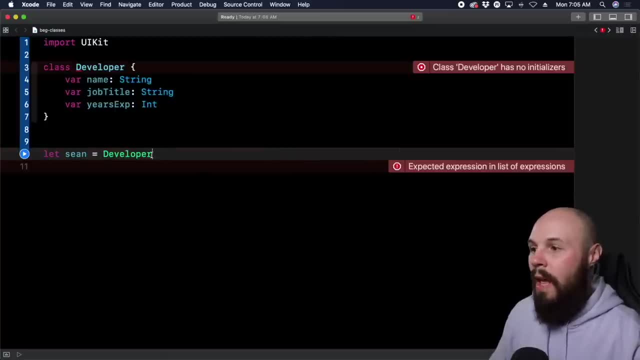 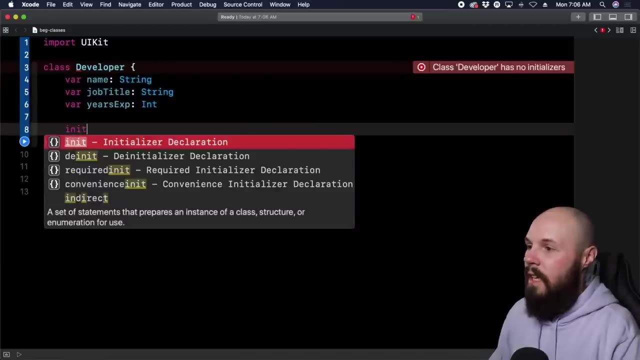 initializers. yet we have to to create that because we have to tell xcode how to create a developer like: how do we build that? so to do that, we have to create our initializer like this: uh, init and the parameters it takes in. it's going to take in the initializer and it's going to take in the. 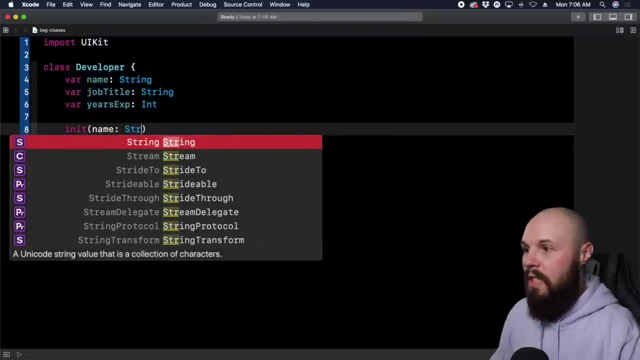 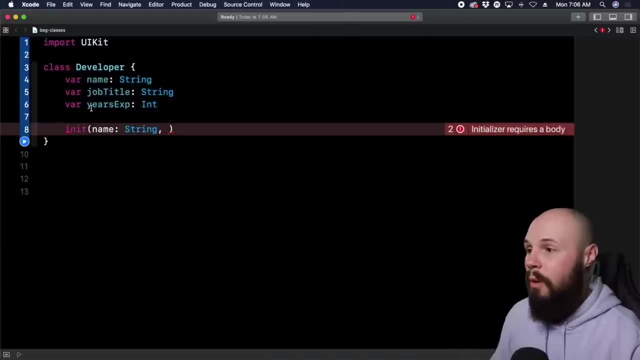 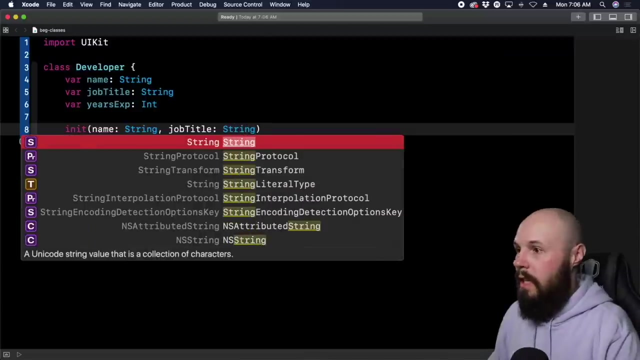 name, and that is of type string and the parameters it takes in are what you want to initialize the values to right. so we want to pass in a name, we want to pass in a job title, we want to pass in number of years experience. so here you go: uh, job title, and that is a string. and now years exp, which? 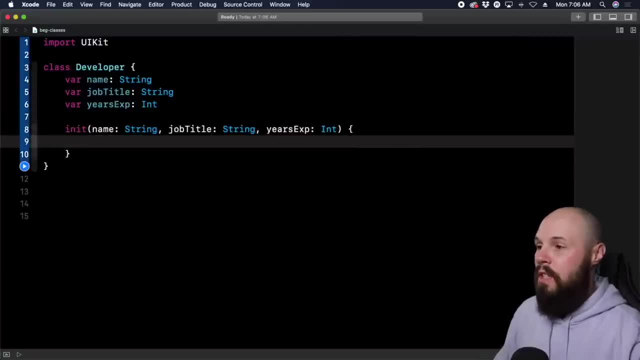 is a int integer, right? so now this function, just like before, we have to set the values that we pass into this initializer, right, because we're going to pass in a string for the name, we're going to pass in a string for the job title, we're going to pass in, you know, an int for the years experience. 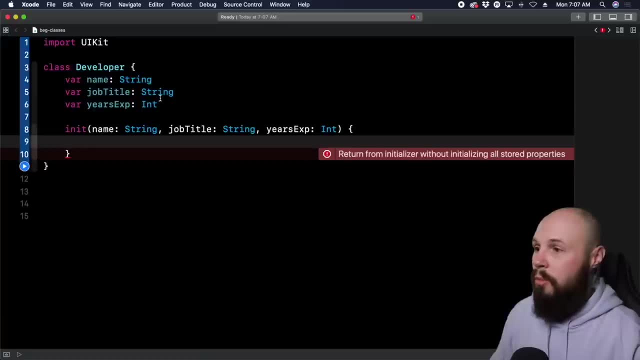 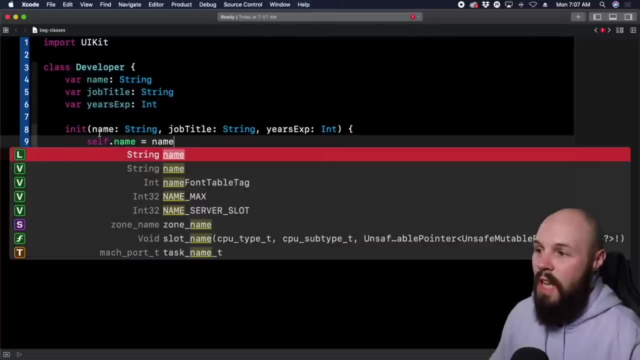 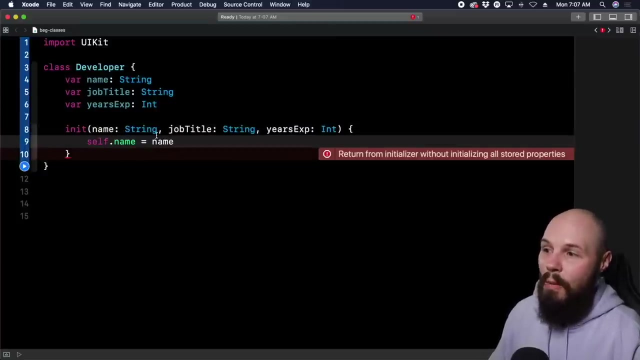 we have to set those to our developers, uh, properties. so here we need self selfname. remember before how we have to distinguish between this name that we're passing in and the developer's name that we're setting. so what we're saying right here is: hey, take this name that we 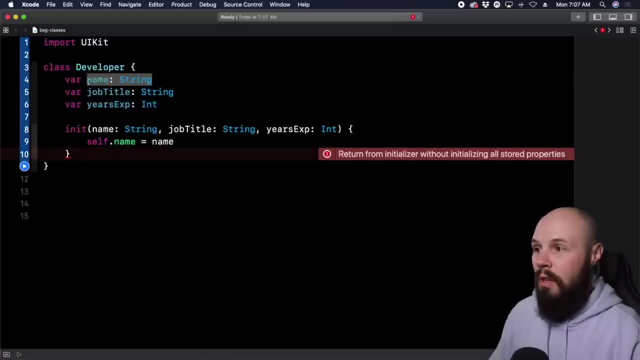 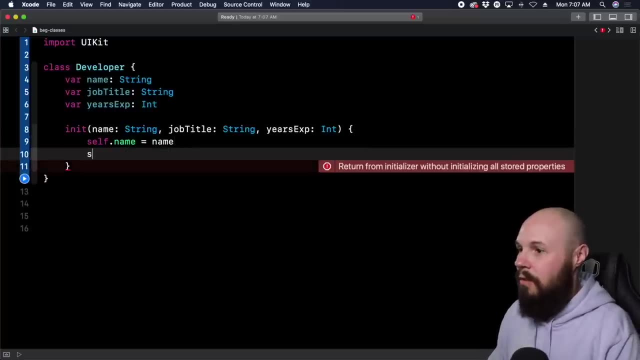 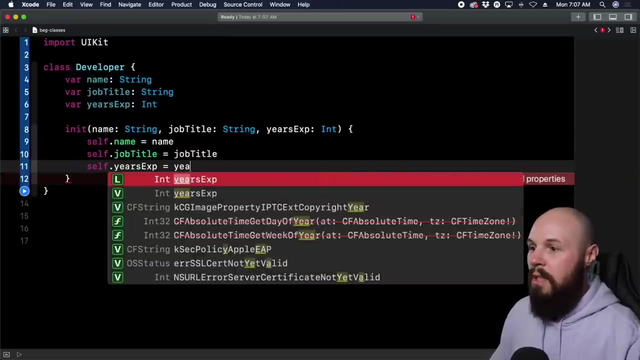 pass in this string and set it equal to my developer's self. we're essentially naming our developer like our developer's being born and we're giving it a name. so very similar stuff here: selfjobtitle equals job title and selfyears exp equals years exp, and. 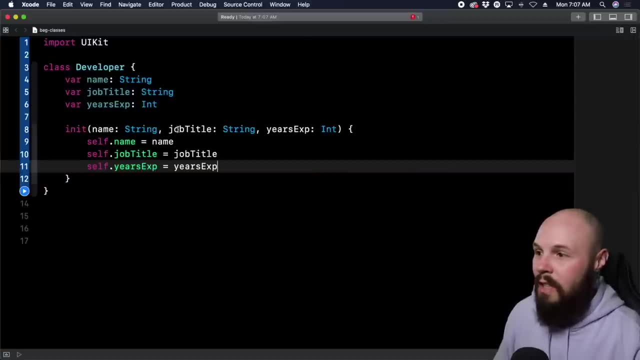 again. the ones in white are the whatever we're passing in. the ones in green are the actual developers properties that we're setting. i know i've repeated myself a bunch there, but uh, this confuses a lot of people so i really wanted to again drive that point home. i know i've said that. 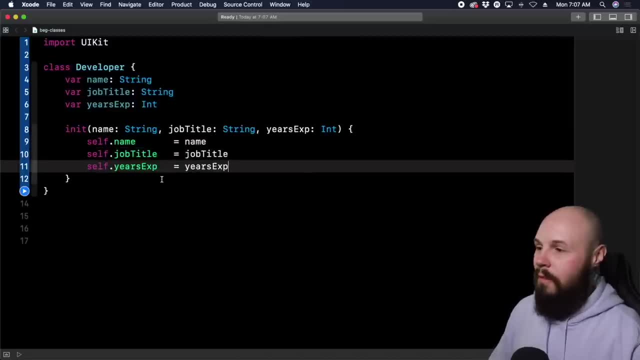 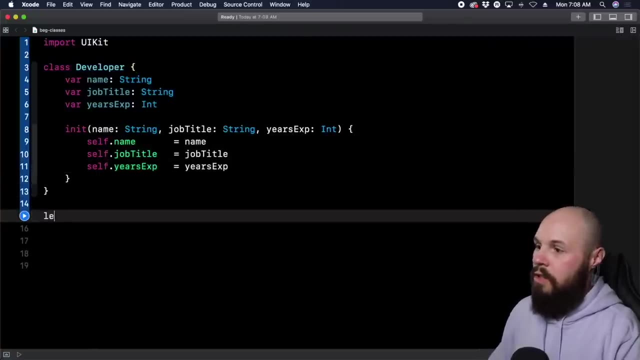 a thousand times too. i like to line up my equal signs. i think it looks nice. you don't have to do that. so anyway, we have our initializer now. so now when we create our shawn object here. so let shawn equal developer and we do our open. 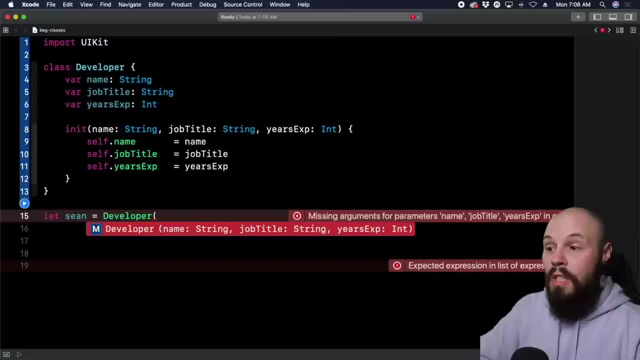 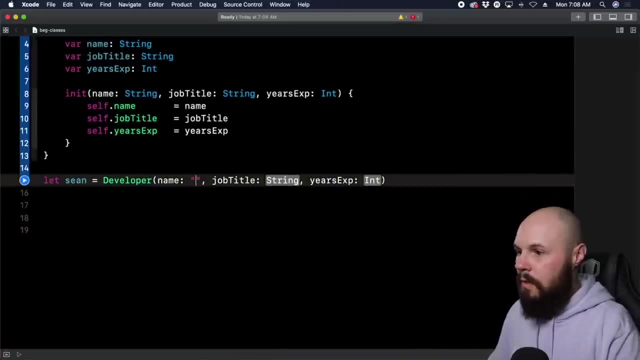 parentheses. you see, we get our initializer, that auto completed, like that's what we just created up there on line eight. so if i hit return now, it'll tell me: okay, pass in a string. so my name is shawn, my job title is ios engineer. years of experience: five right. so now i have this object. 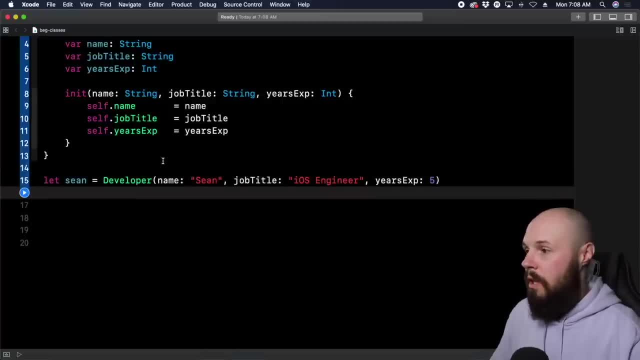 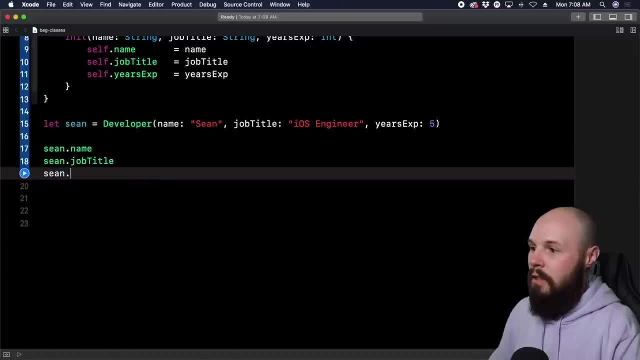 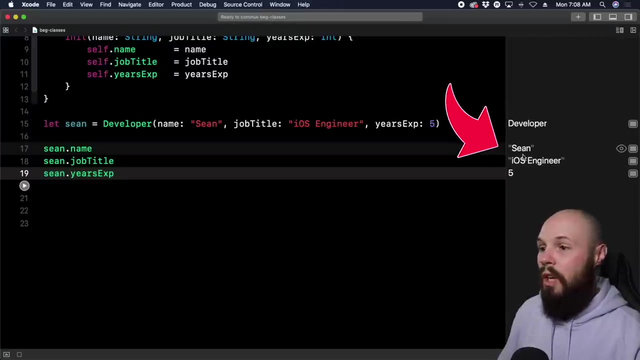 and now shawn has all these properties. so right, so if i do, uh, let's see shawn dot name. shawn dot job title: shawn dot uh years exp. and then i run it. you're going to see over here on the right, look, the value of shawn dot name is shawn. the value of shawn dot job title: ios engineer. 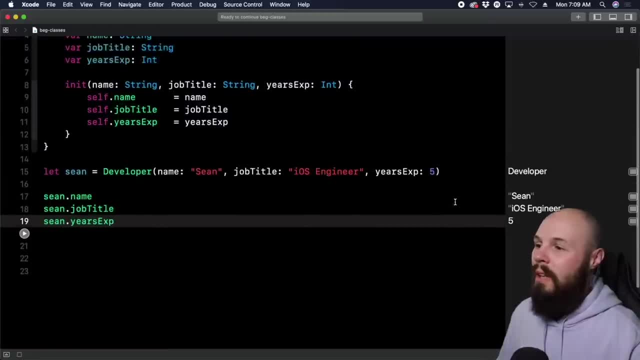 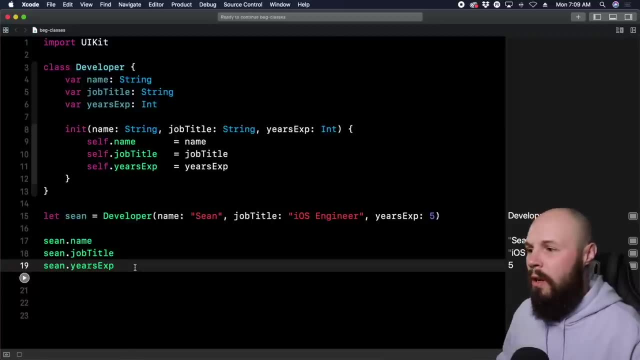 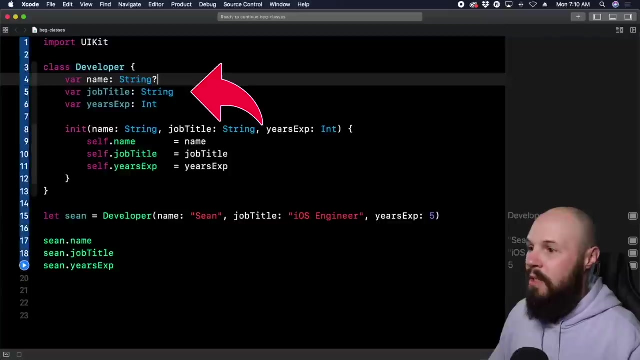 shawn dot years experience: five. so that's the basic way to set up a class with an initializer. now there are other ways to initialize classes. uh, another common one is you just want an empty version of it where name, job title, years, experience are nil. so in order to do that, we need to make these optional, our properties up here. so string is: 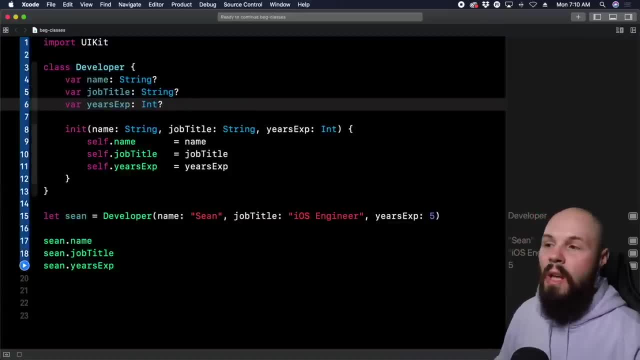 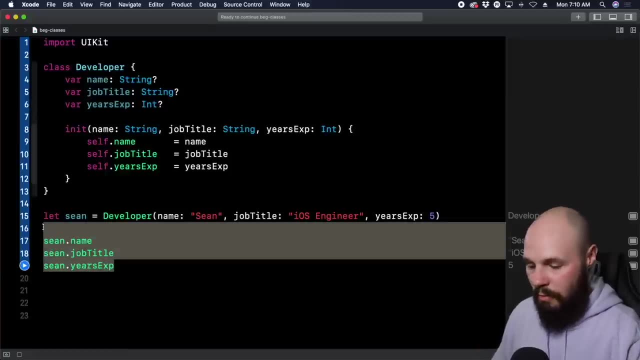 optional. uh. job title optional, years experience optional. by making these optional, we can create an initializer that just creates an empty developer. uh, let me show you what i'm talking about. let me get rid of my shawn one right here, and we have to create this init here. that is the 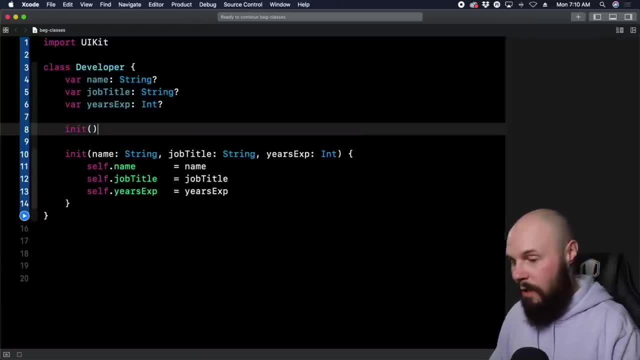 empty one, so init no parameters, we're not passing anything in, and then we do open and close curly braces because we're not doing anything. we're just initializing the empty uh developer here, so that allows us to do something like this. so let shawn equal developer and then just an empty initializer. 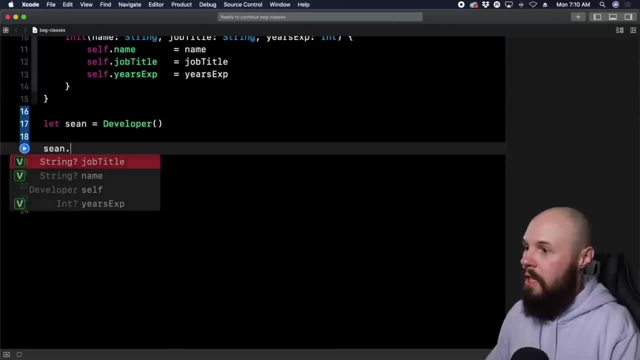 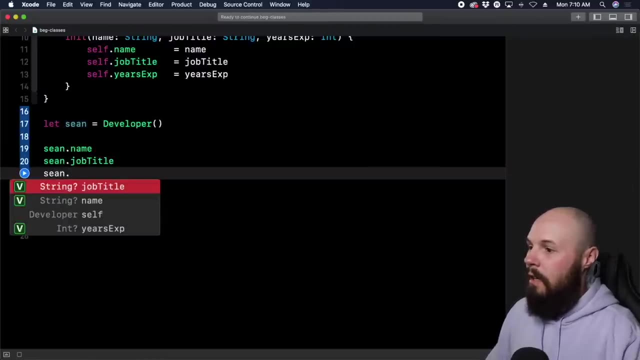 so now let's go down here and if i do shawn dot name, you see it's an optional shawn dot job title. see, that question mark makes it an optional shawn dot. uh, years experience, by the way, this dot is called dot syntax. uh, just a little side note, um, so now when i run it, i'm going to be able to do. 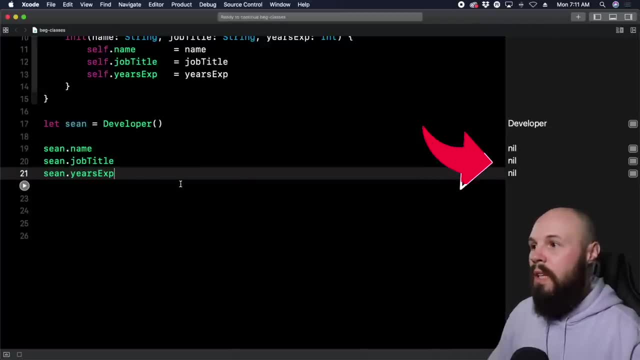 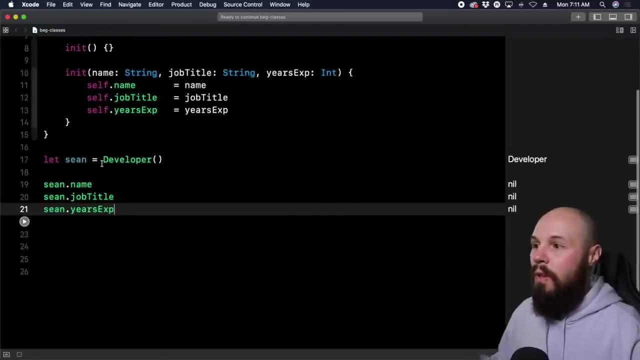 it. you're going to see all these values are nil. there you go: nil, nil, nil, nil. but because i've made them optional, it allows me the flexibility to create an empty one and then i can add those properties later. right with this initializer. all those properties were set when the object was. 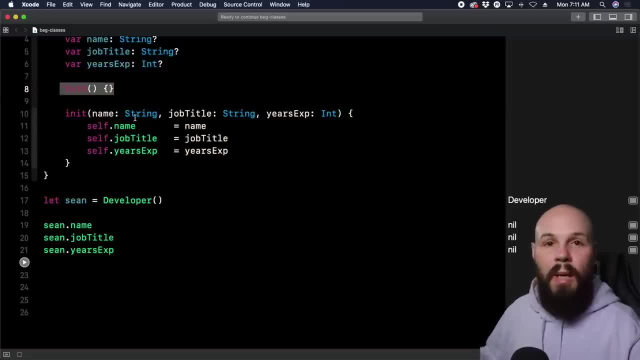 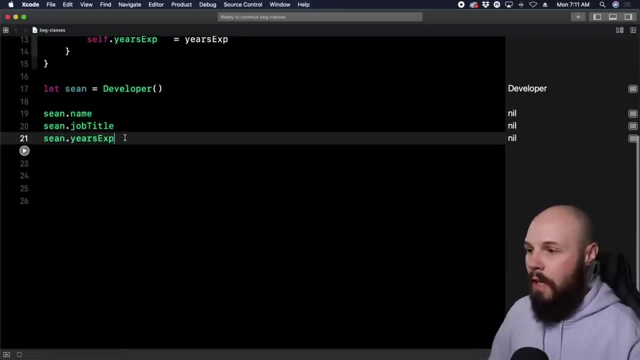 created. by doing it this way, uh, with just the empty initializer, we're creating the object. uh, that is empty, essentially, right. all the values are nil. but we can change those uh later, right? i can do. uh, shawn dot name equals uh, you know, joe, and then i can add those properties later, right? so 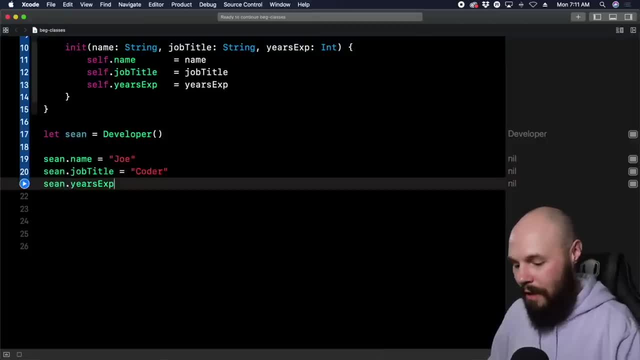 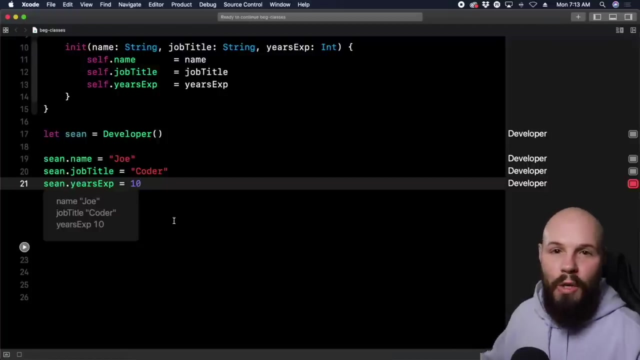 uh, shawn dot. job title equals coder. years experience equals, you know, 10. so now when i run it, uh, it's going to have value now. so if i open up this developer here you can see it'll say name: joe. job title: coder. years experience: 10. so by initializing the empty one you can set the values. 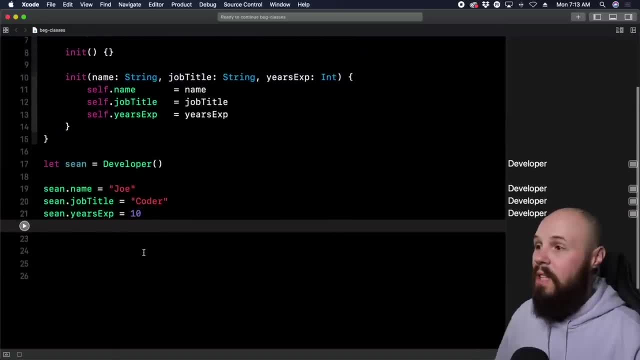 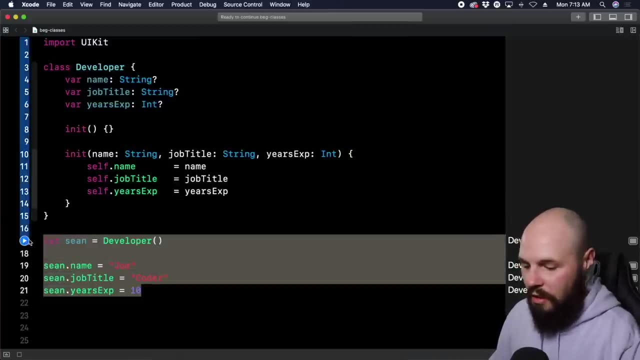 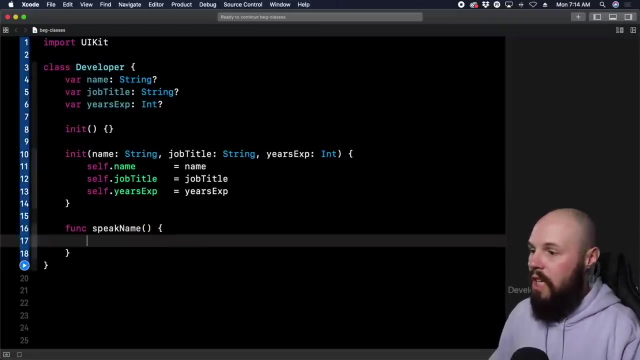 later if you need that flexibility, uh, in your code now, aside from properties, classes can also have functions and functionality. so here in our developer class, let me just get rid of this here. uh, we'll do, we'll create a function- func speak name- and that gives us some functionality here. 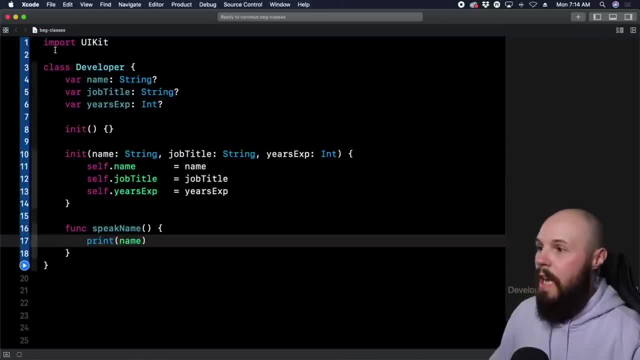 and we can do print name, which is our name, up here on line four, that we assign it now. again, if we uh assign it with an empty initializer, it's going to be nil. so if we create our shawn developer again- i'm just again reinforcement here- the shawn equal developer, and we see, now we have the empty. 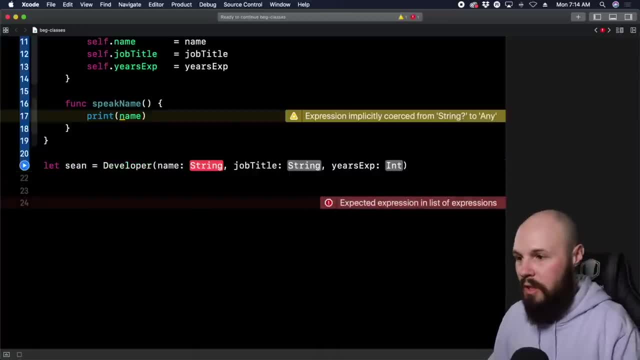 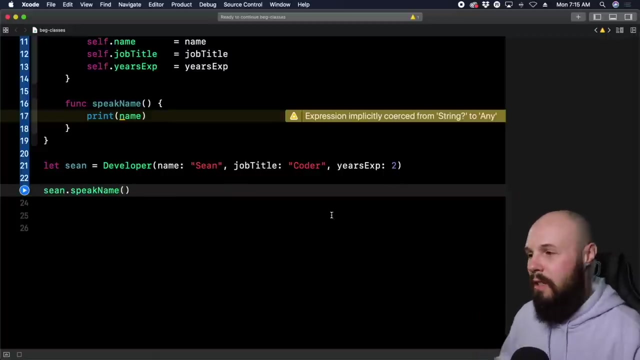 initializer or the ones that we want to pass in. we actually want to pass in values here. so again, shawn job title: uh, coder, just for short. and then two years experience. so now i can also do seanspeak name right, i put some functionality onto this class and if i run this, uh, you're. 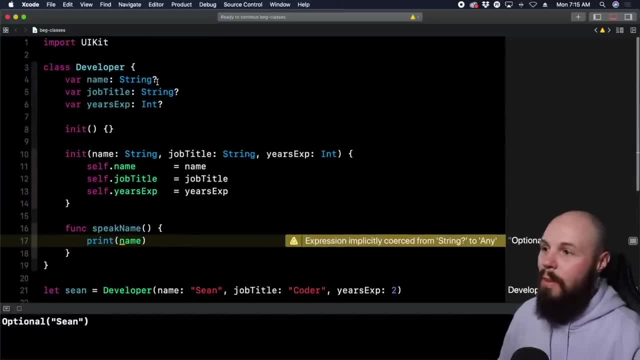 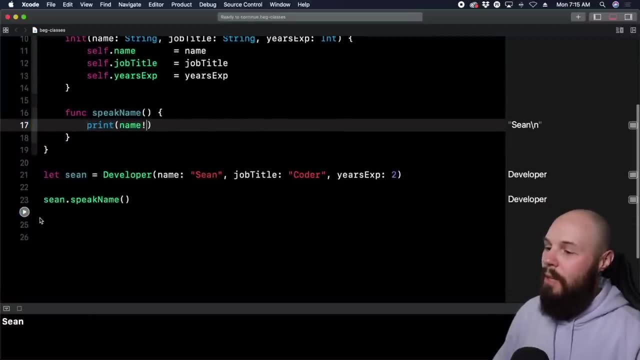 going to see. it's going to print: well, optional sean- again. that's because name up here is an optional- uh force unwrap again. remember that's the dangerous one, but we're just doing this real quick. i don't want to go through the full unwrapping now it just prints: uh, sean, and. 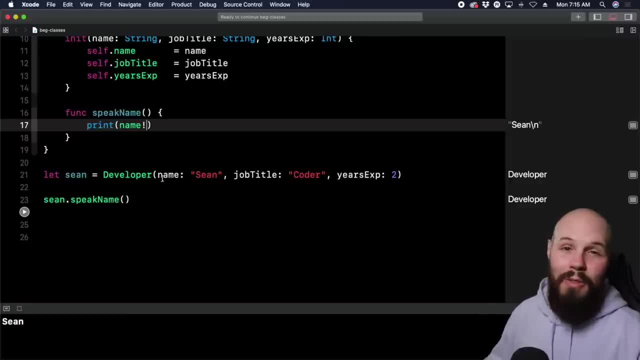 what i just said. i don't want to go through the full unwrapping. that is often why you see people force unwrap. um, it's a shortcut, it's kind of the lazy way, um, but i wanted to illustrate that to show that that's how force unwraps usually end up in code bases. um, anyway, a little side note, but uh, 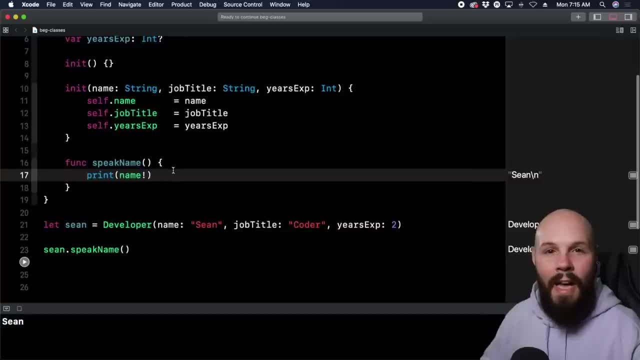 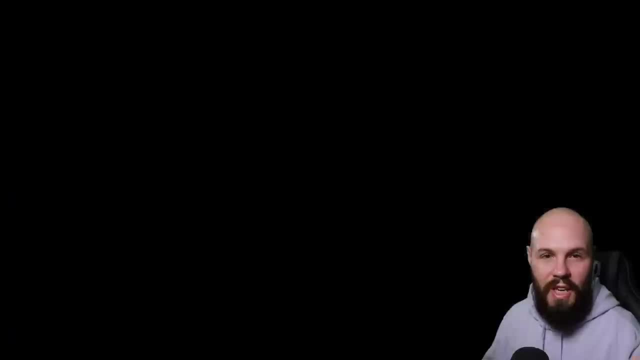 that is the basics of creating a, a object, a class. now a struct is another kind of object that we're going to get into in another video, but the reason i'm mentioning that is because i want to show you this in action. here is our user object, again from my github followers, course. 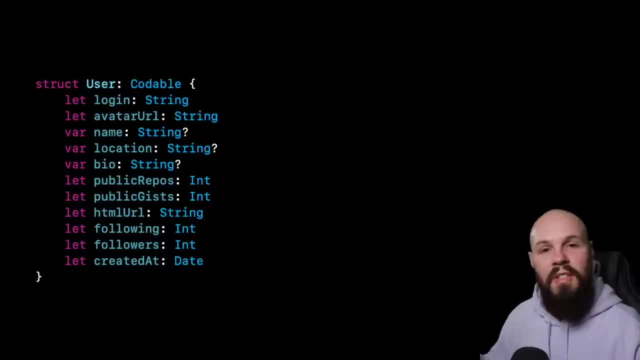 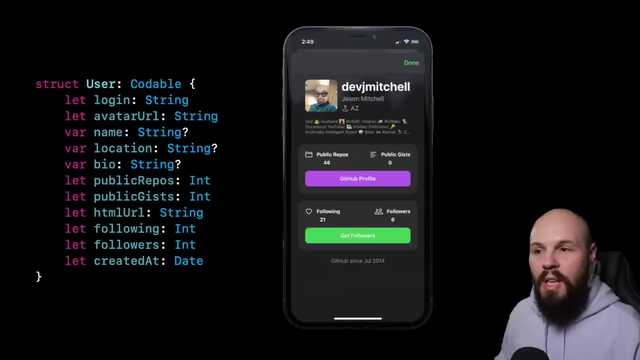 and, as you can see, that is a struct, but you can see all the properties, very similar to what we did with our class. but the reason i'm showing you this is because i want to show you the screen right next to it, to show you this object in action and how it's actually being used. 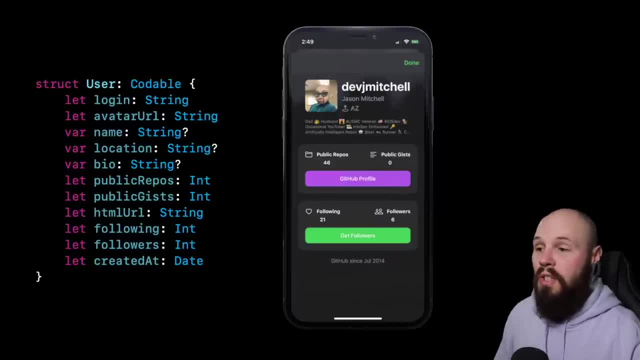 so let's look at this. right like, our user has a login. that's what we're using for this name. right here, our user has an avatar url. that's what we're using to pull down the image for the avatar that you see. here we have name, location, bio, right, how many public repos, public gist, uh, etc. so you can. 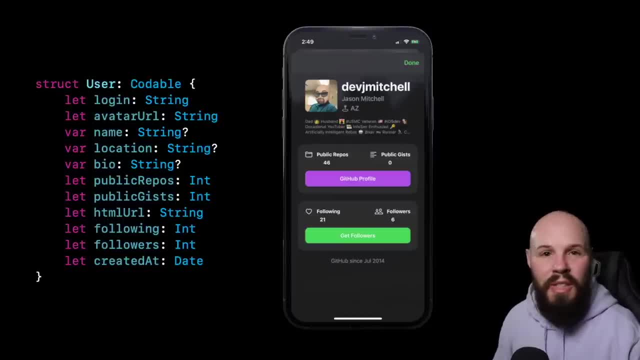 see, here's an example of an object and you can see how we're using that object to populate this into the screen in our class. so let's look at this from the third video. so we're going to show you demo and we're going to show you very briefly the process of how we can use this. 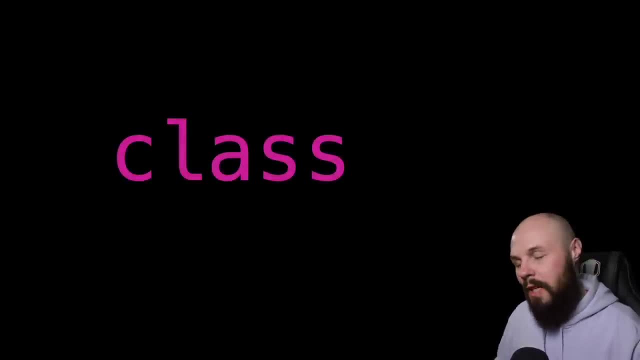 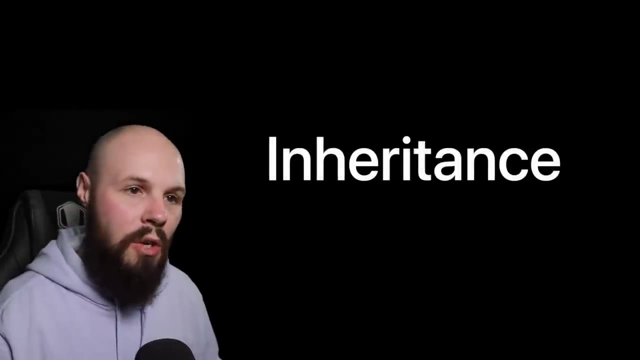 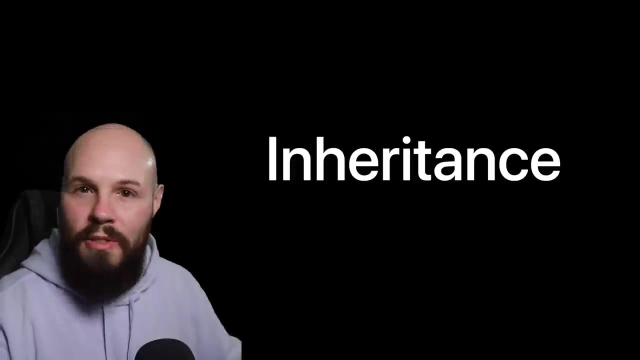 to populate this uh visual image on the screen with that data. so we'll leave it at that, showing it in action. let's talk about inheritance, because that's a big thing with classes, and then we'll move on to structs and reference types and value types, as i mentioned at the very end of the last. 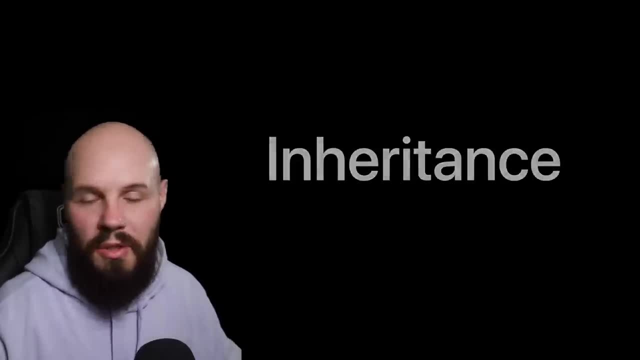 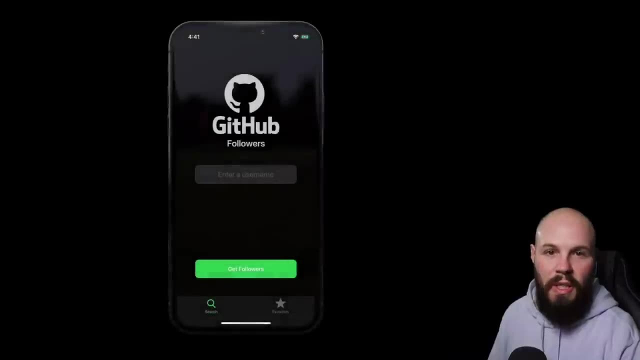 video classes can be subclassed, which means they also have inheritance, so that subclass That. here is a custom button that's been created again in the GitHub followers course. Here's what the button looks like on screen. It's the green one at the bottom. 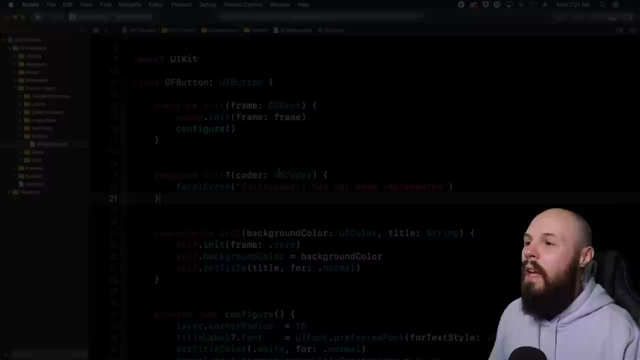 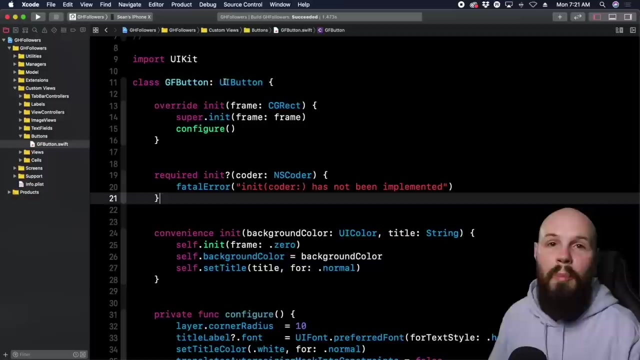 You see how it has rounded corners. you know big bold text. Well, here that is a class called GF button and you can see it is a subclass of UI button. That's what this colon UI button means. So again, this reads as the class is a GF button, which is a subclass of UI button. 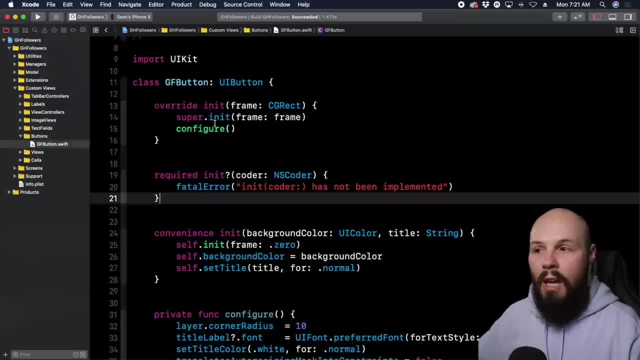 So what that means for us is we're getting all the features and functionality of iOS built in UI button right By default. iOS has a button has all the push, the tap functionality, all the stuff you would expect a button to do. iOS has done for you. 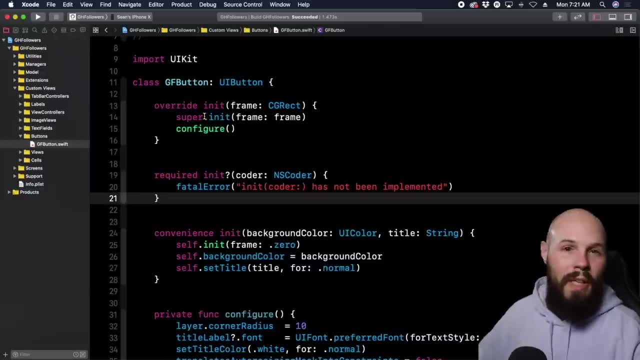 What we're doing is we're subclassing that into a GF button, So again we get all the features of the superclass or the parent class. you'll hear it called this UI button. However, we want to give it our own little custom feel and functionality. 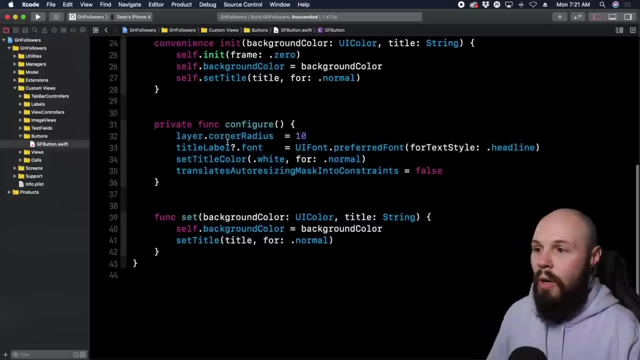 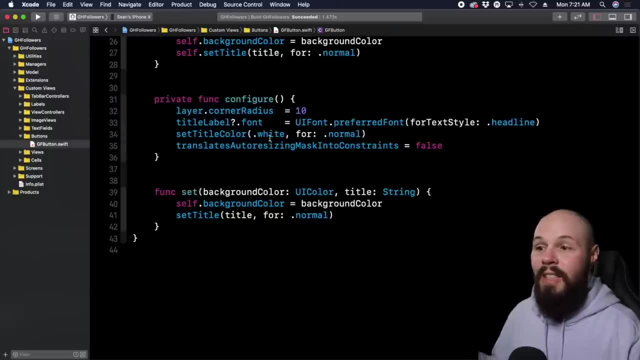 So down here, that's what we're doing. You can see I have a configure function where I'm giving it a corner radius, which is the rounded corners of 10.. You can see I'm making the font A specific font type, I'm setting the title color to white and then we're doing some. 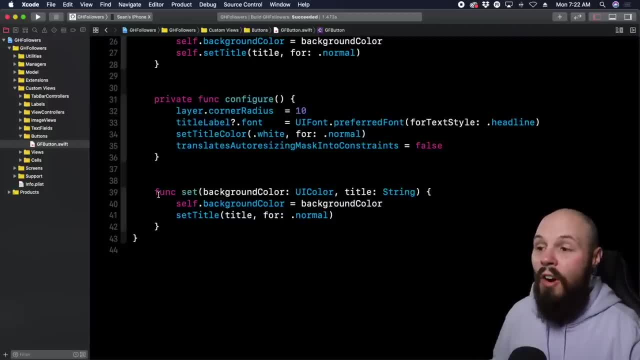 auto layout stuff. more on that in a bit. And then you can see we gave it a function as well where I can call on my GF button. I can call set background color and title. So this allows me to quickly change the background color to whatever I want and also pass in. 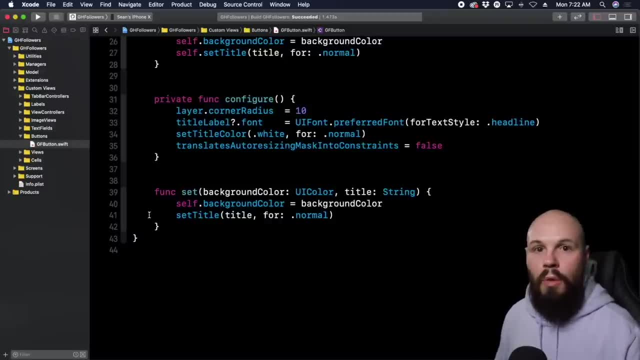 a title. You know whether I want it to be get followers or, you know, go to the repo. whatever I want the button title to be, I can quickly pass that in. So we're going to build on our developer example to show it to you in action. but I wanted 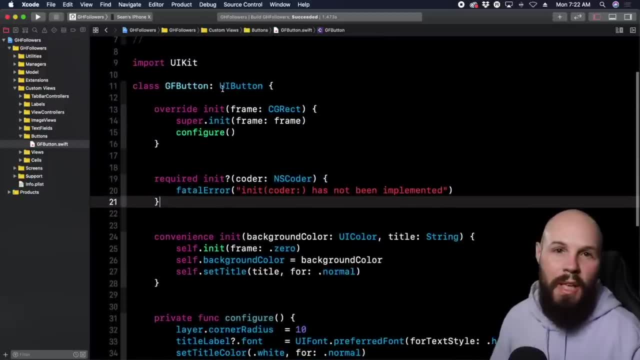 to show you like kind of a real life one. Again, the GF button is a subclass of a UI button and you'll see that a lot in UIKit, For example, when you make your own view controllers. let's go to that there. screens our search. 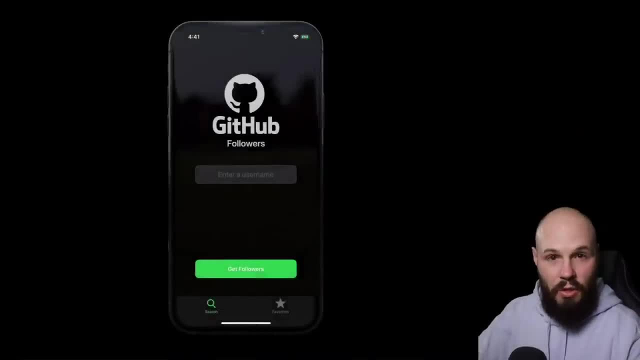 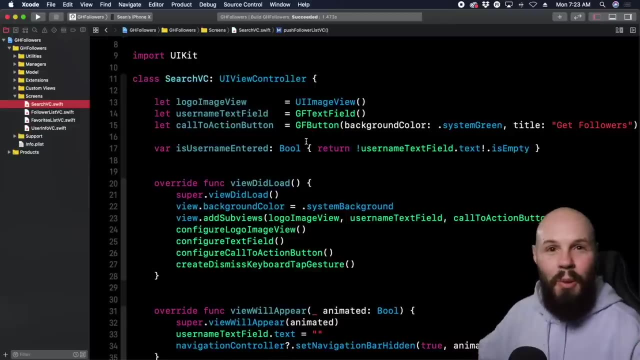 VC, So our search view controller, which, again, is this what you see on the screen, our initial screen. here is a subclass of UI view controller. So again, we're getting all of iOS's built in UI view controller, which is the screen. 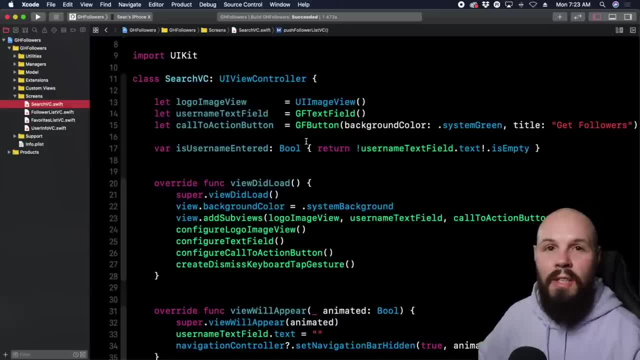 We're just making it our own. So again, that's subclassing and inheritance. We're going to go ahead and do that. Let's build our own version. We're going to create a subclass of our developer. but let's clean up a little bit from our previous. 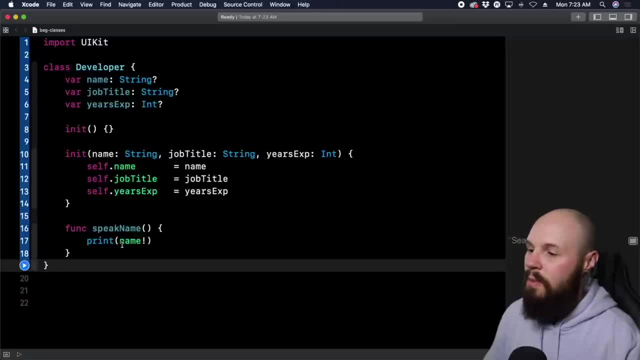 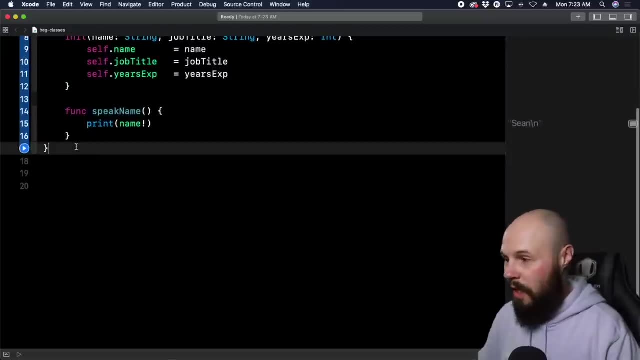 playground here. Let's get rid of. no, we'll keep speak name. We'll get rid of this initializer because we're not going to initialize an empty one. I'm just making space here, Okay, So down here we're going to create another class, class called iOS developer, which is 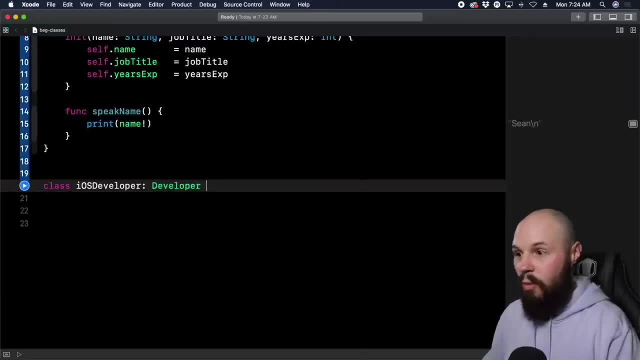 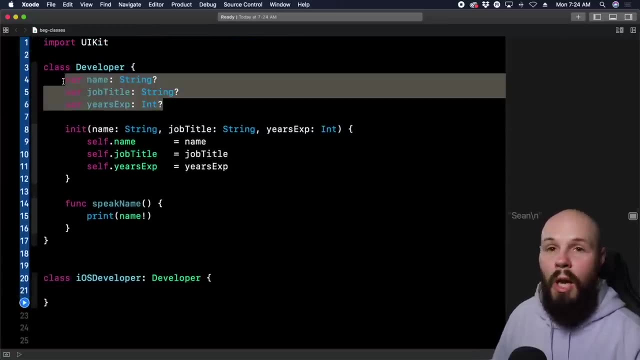 a subclass of developer, right. So what we're saying here is: give me all this functionality up here and properties. So my iOS developer. It's automatically going to have a name, a job title, years experience. My iOS developer is going to be able to speak its name. 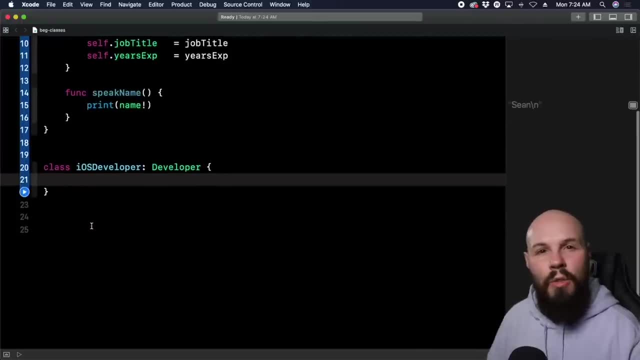 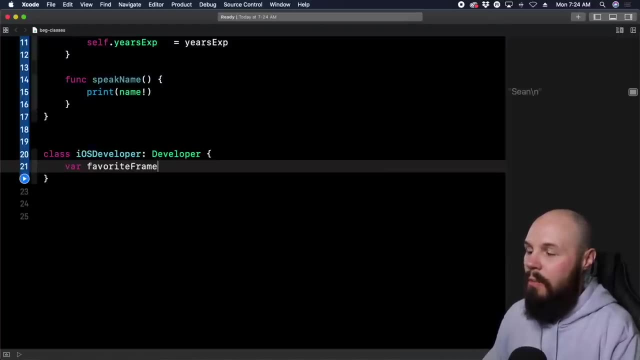 Like it's going to get that automatically. However, we want to add like our own special things to our an iOS developer, So maybe we want to add a property called a favorite frame work and that would be a string. it's optional. 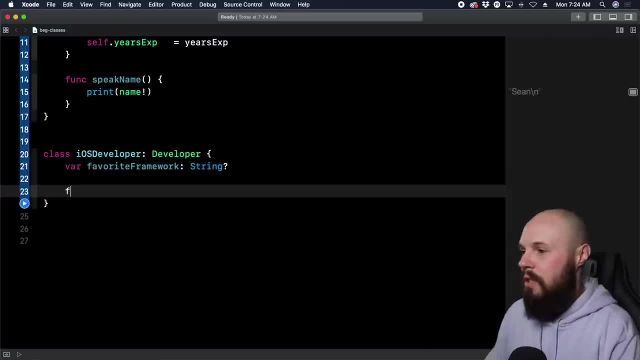 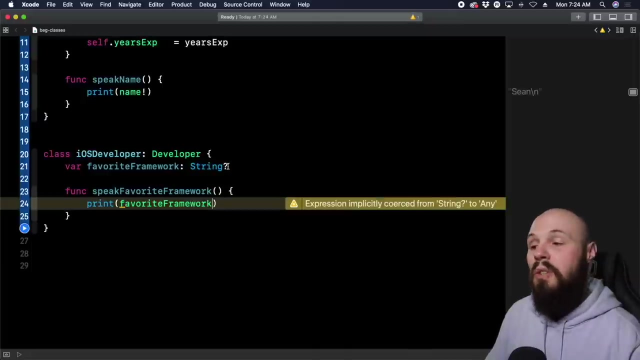 And then maybe we want to speak that favorite framework. So funk, speak favorite frame, work, Okay, And that will do print favorite framework. And then you see it is an optional, so it could potentially print nil, or it could print the framework, And you know what? 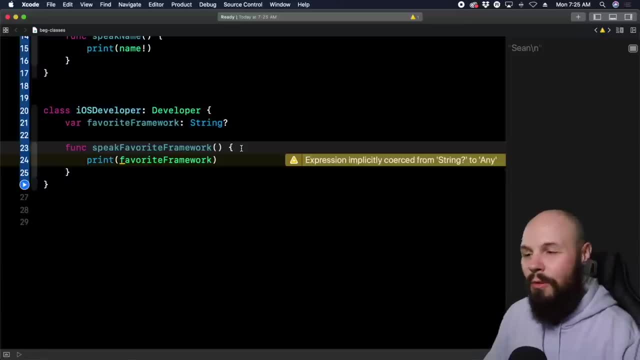 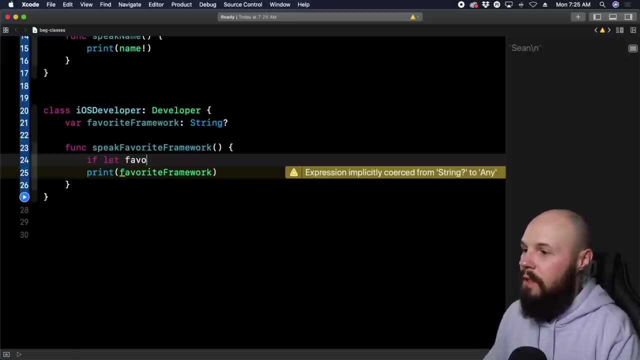 Let's actually do a little exercise in the unwrapping member. I said last time I'm going to be lazy and force unwrap it. Let's actually do it for real, to show you an example here. So what we could do here is if let favorite frame work. this is us creating new variable. 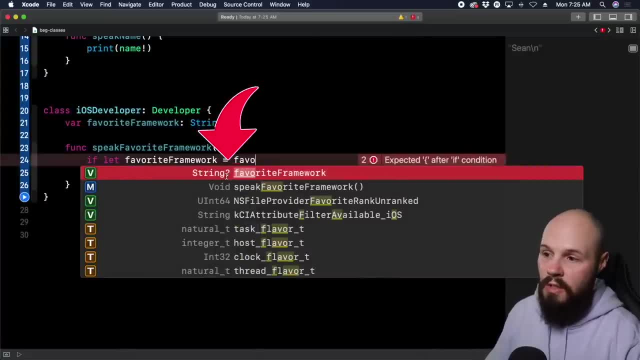 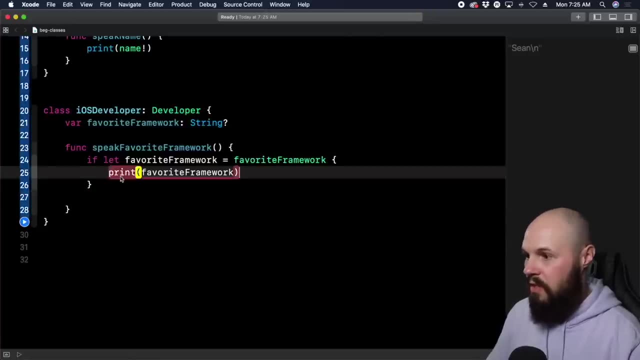 equals favorite framework. You see, So if we're going to print that optional one cause it says that, uh, then we do this, we will print. I'm going to cut and paste this here: print favorite framework and you see it switched. 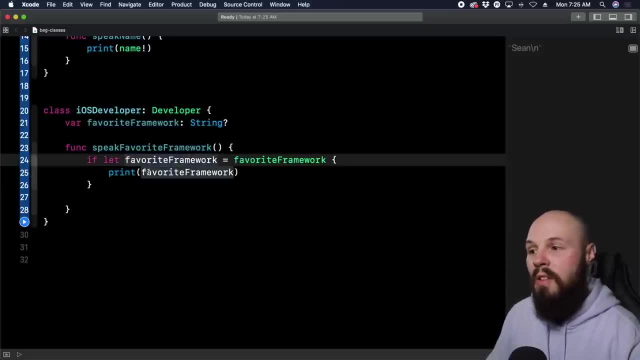 to white. So that means this is this one. Remember Cause this is the variable we said that we can use within scope. So what we're saying here by unwrapping that optional is: if favorite framework, uh, I'm sorry, if this favorite framework has a value, set it equal to this variable: favorite framework. 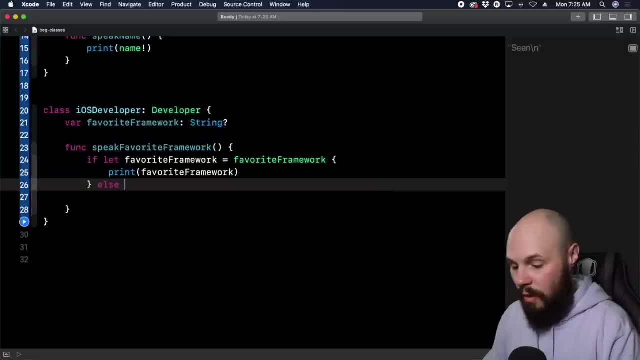 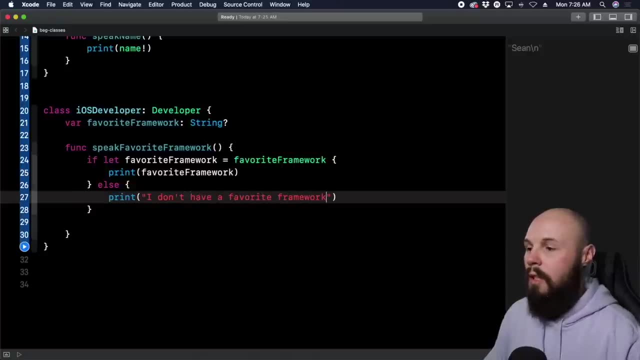 and then now use this favorite framework to print that else. So this is when it's nil We're going to print. I don't have a favorite frame work right, So that that is a how you should actually unwrap the optional there. 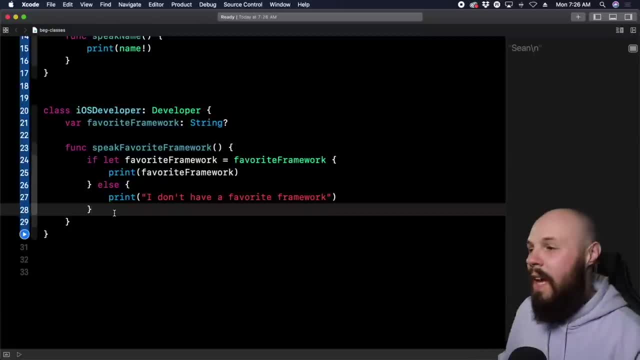 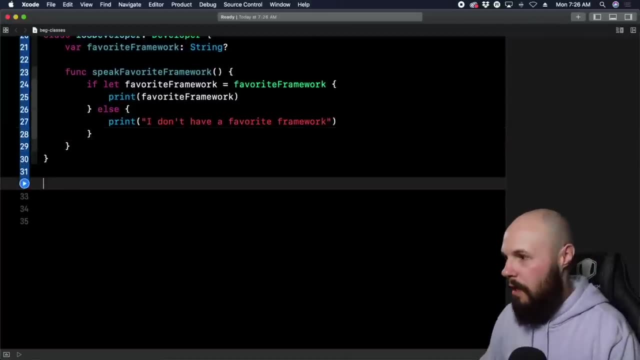 So now you can kind of see why sometimes developers get lazy. They don't want to go through that. Um, don't be lazy. So now let's create, uh, Sean as an iOS developer. Um, so let's do that. uh, let Sean equal iOS developer. 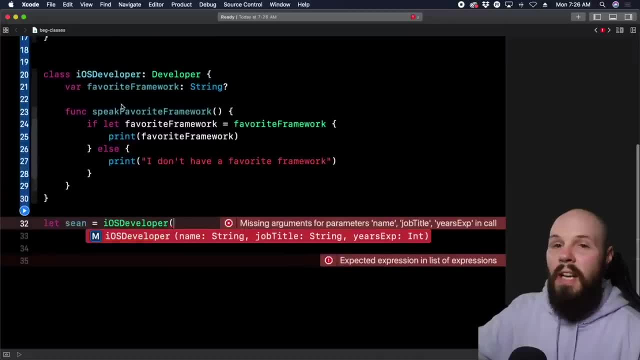 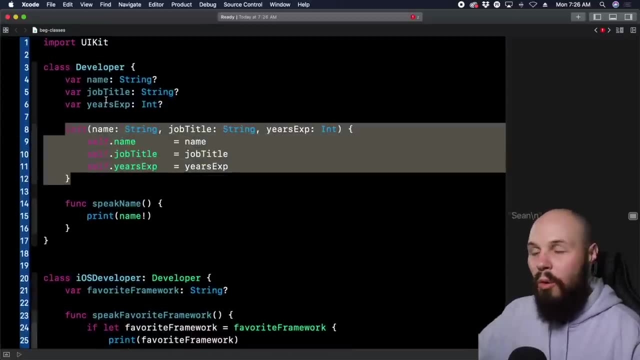 And now the initializer. see, I get the initializer right. We didn't set an initializer in our iOS developer subclass. Okay, I get this initializer up here from developer because again, we're inheriting all those features and functionality. That's the power of inheritance. 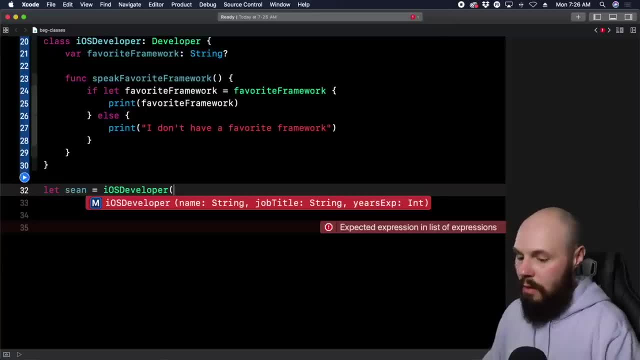 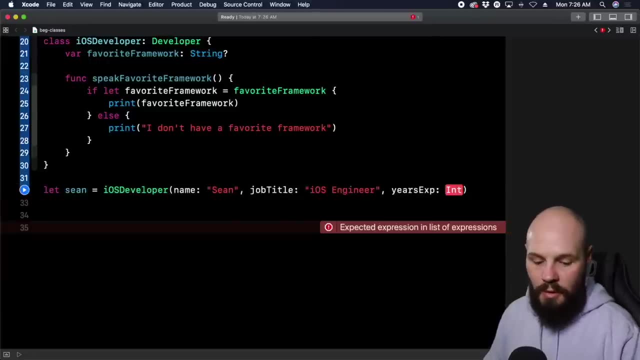 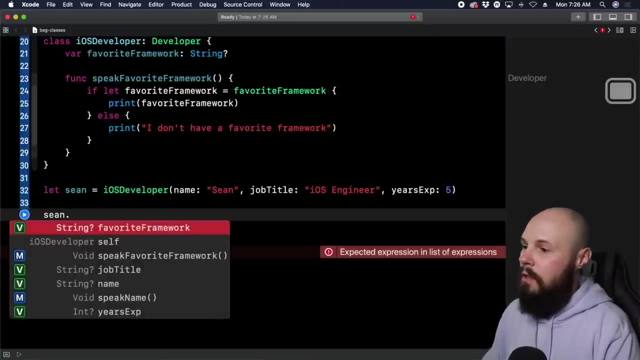 So, iOS developer: uh, let's do this here. Name is Sean. job title: iOS engineer. your experience five, But now we will do uh Sean dot. well, no, let's, let's do uh Sean dot. speak a favorite. 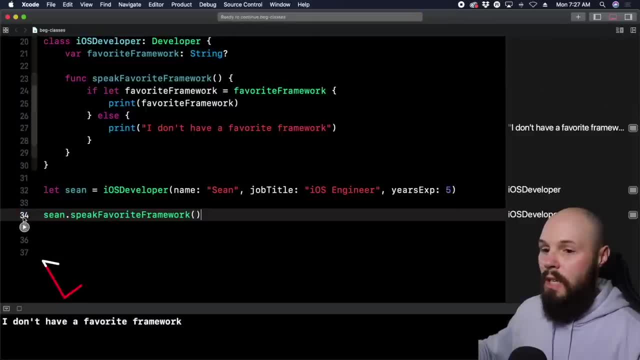 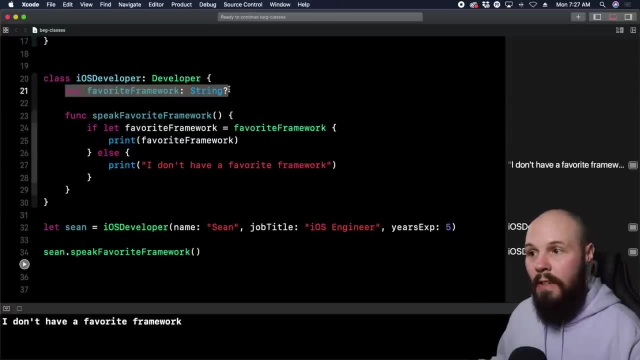 framework. We haven't set the favorite framework yet, So let's run this and it should say: I don't have a favorite framework, That's because up here, favorite framework was nil, because we never set it again. That's the power of being an optional. 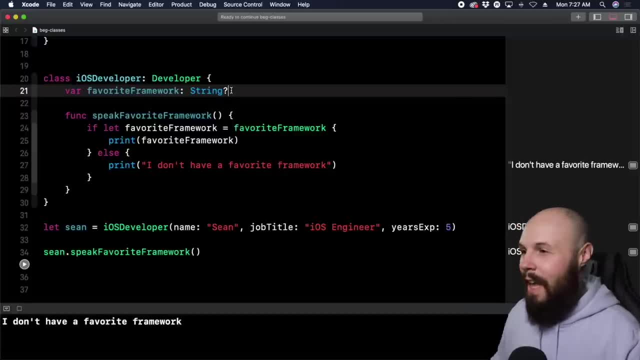 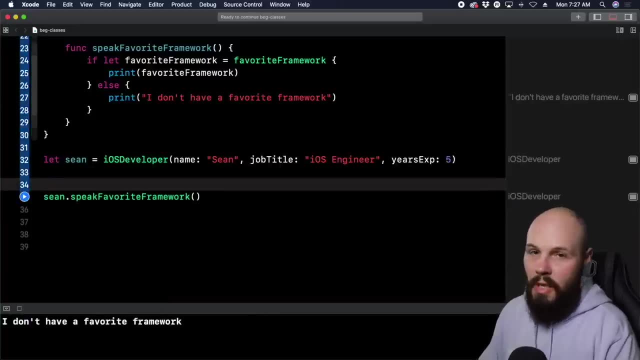 You can see why it's called optional: because you have the option to have it or, like, not have that value. So now let's actually give it a value. So, Sean, well, above speaker, favorite framework. So we set it and then speak it. 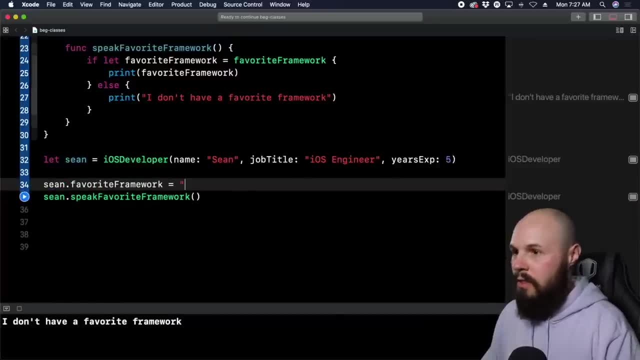 So Sean dot favorite framework equals: uh, this is a string, right, We'll call it AR kit. That's not really true. I don't have experience with AR kit yet, but Hey, It's the first one I thought of. 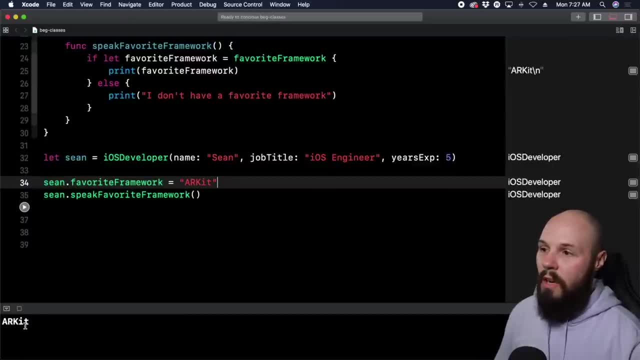 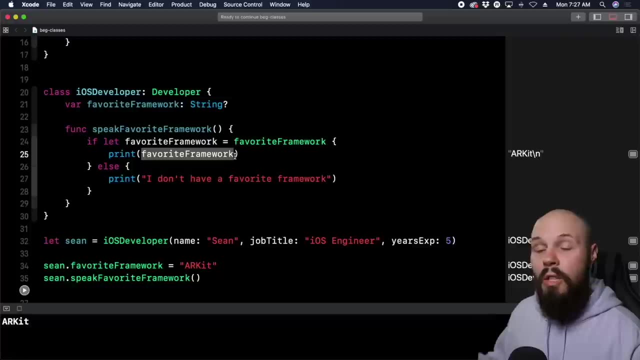 So now when we run it, Sean speak favorite framework. you see it speaks AR kit. And again back up here to to reinforce the concept of optionals, because we unwrap the optional and it had a value. We use it here and we printed that favorite framework. 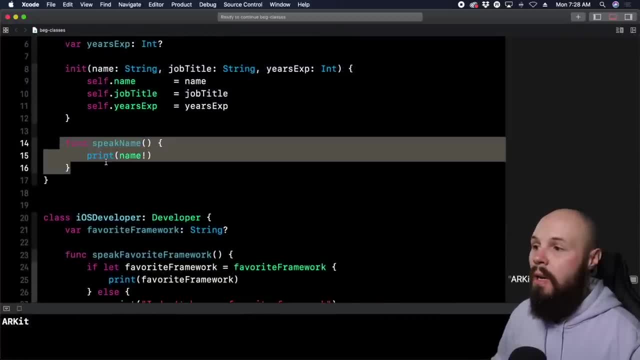 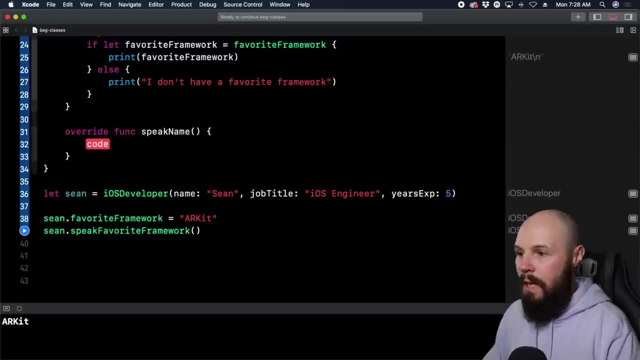 Now you'll notice up here: speak name. Our iOS developer has this: speak name uh, functionality uh. but we can also do what's called override, So this is where so override, speak name Uh. so now this is where you can say like: yes, I know. 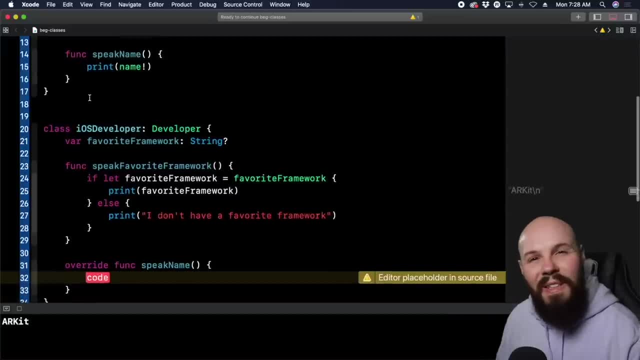 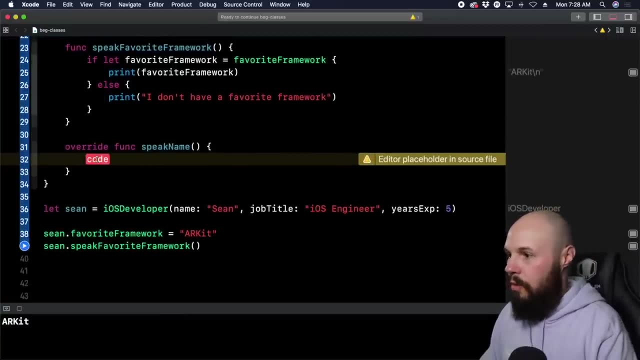 I have this speak name functionality as a subclass, but I want to do something a little different with that speak name. Uh, so this is where you override that speak name function. Uh, so you can do, I would do like print, let's do name. 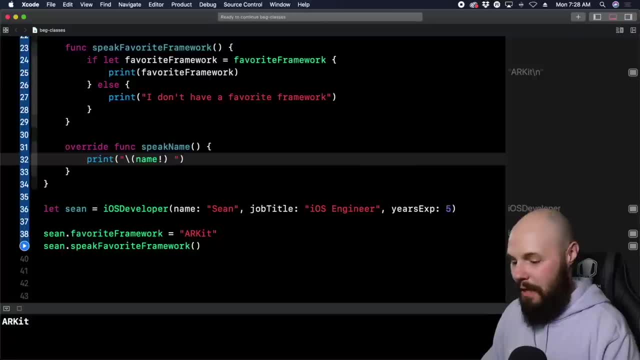 And again we're going to force unwrap cause we're going to be lazy and we'll say: dash iOS, uh name, dash job title. So we want our speak name to also speak our job title, because we're proud to be an iOS developer. 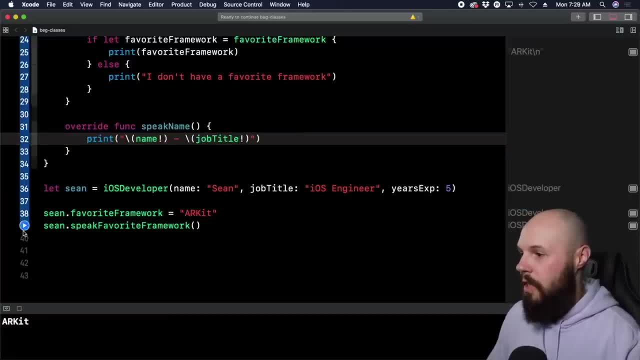 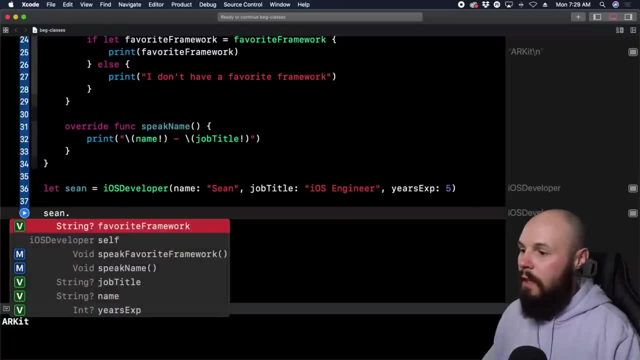 Uh, engineer there, And again we're going to force unwrap that too dangerous living dangerously. So now down here, uh, we've created Sean as an iOS developer. If I do Sean dot, uh, speak name, it's not before. 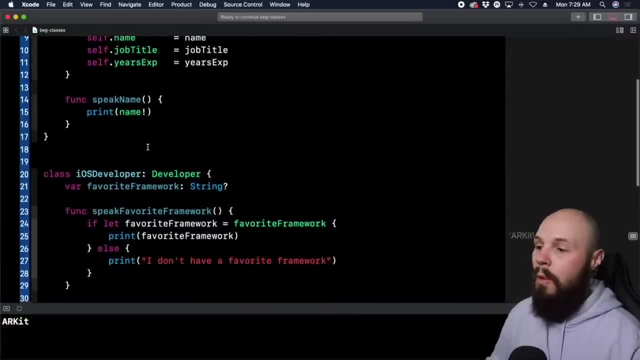 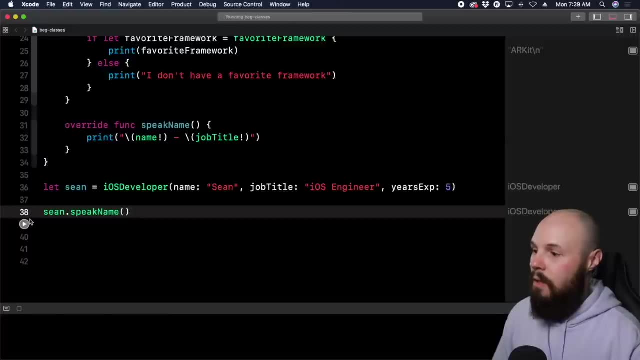 If I wouldn't have overrid that function, it would have just spoke my name. but because we overrode the function and gave it new functionality, Now we're going to speak the name uh dash job title. So down here, Sean dash. iOS engineer. down here, as you can see. 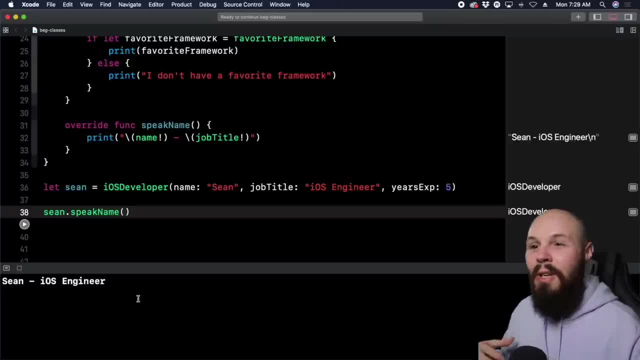 So that is overriding. Uh, This is kind of like inheritance, right? It's kind of like if you're, if your mom and dad gave you blue eyes and you're like, no, no, I don't want blue eyes, I want brown eyes. 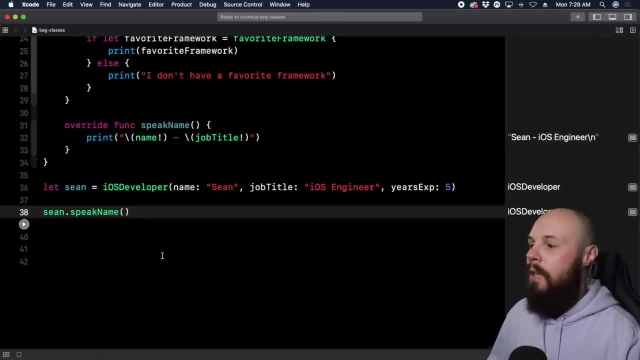 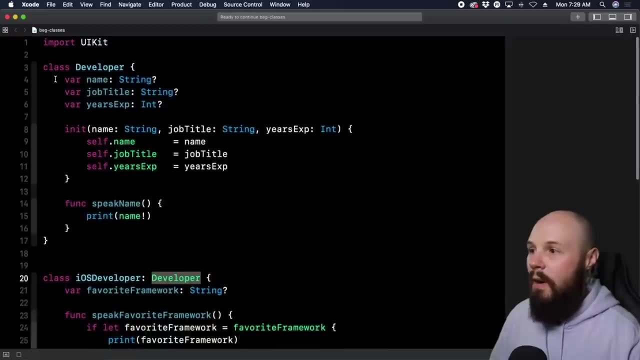 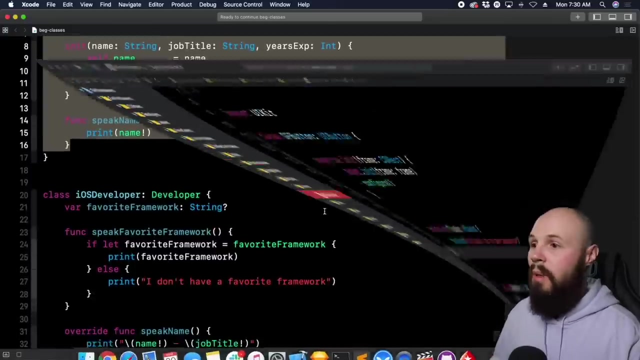 And you override. It is essentially what you're doing here. So again to reiterate: uh, our iOS developer class is a subclass of developer And because of inheritance, we inherit all this functionality of our developer uh, to kind of create our own little custom version of it. again back to the uh GF button example. 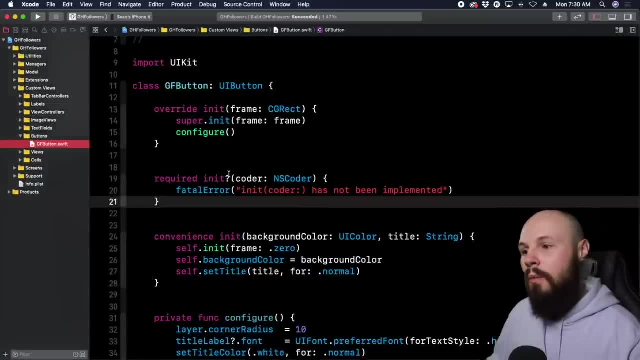 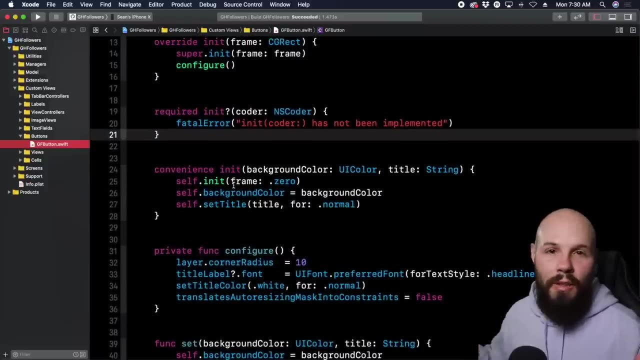 here We get all the functionality of a regular UI button. We just added our own little flair to it, You know, giving it the rounded corners and different font, uh, et cetera. So again, that is the concept of inheritance. 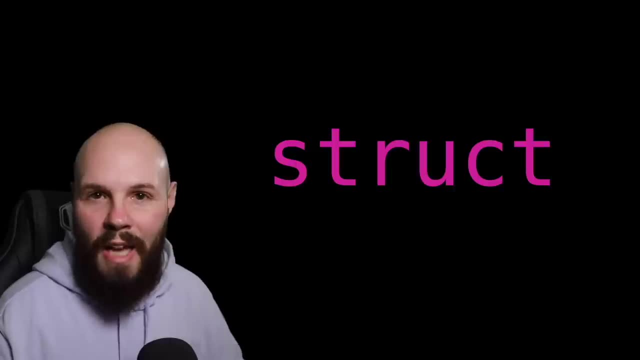 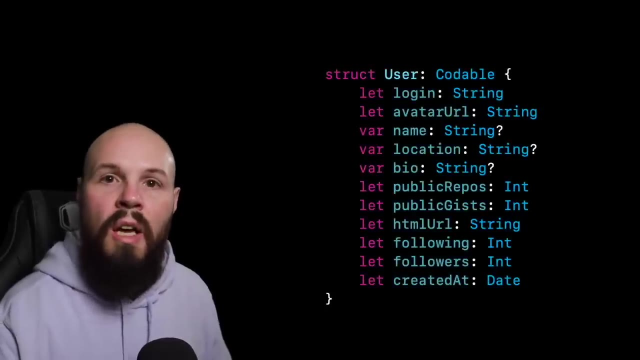 The concept of a struct is actually quite similar to that of a class, in that it's an object, It can have properties, It can have functions. Remember we talked about that user struct from the GitHub followers course? Uh, you know, you see, that has properties as well. 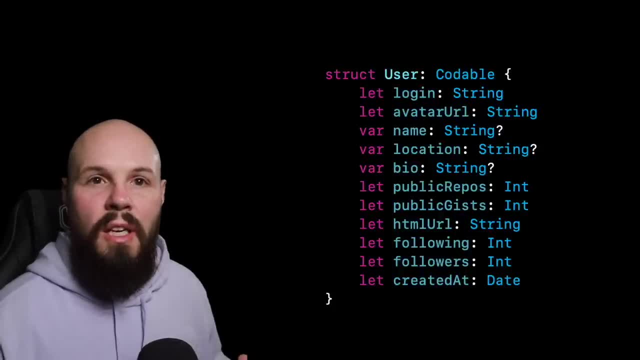 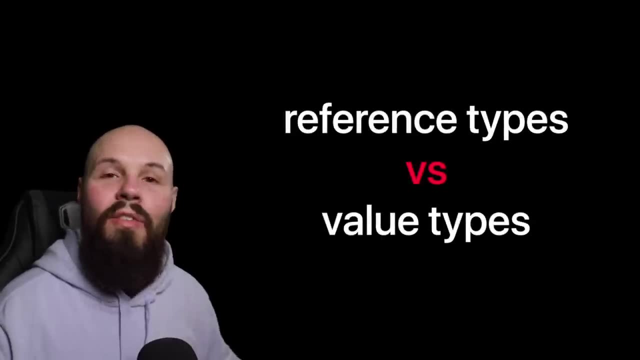 Now, structs are a lot more lightweight and performant than classes, And the reason why is because they are value types. Let's talk about the difference between reference types, which classes are reference types in value types. structs are value types, So a reference type, which again is classes, point to a specific set of data, whereas structs. 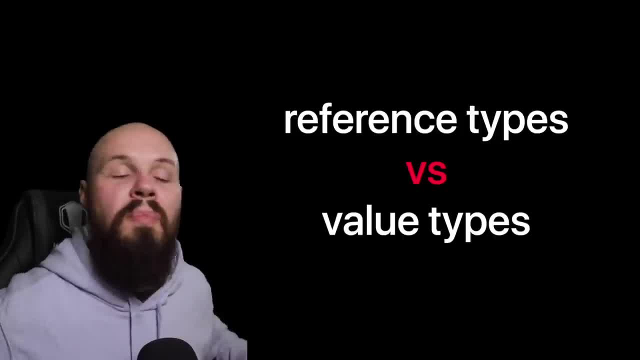 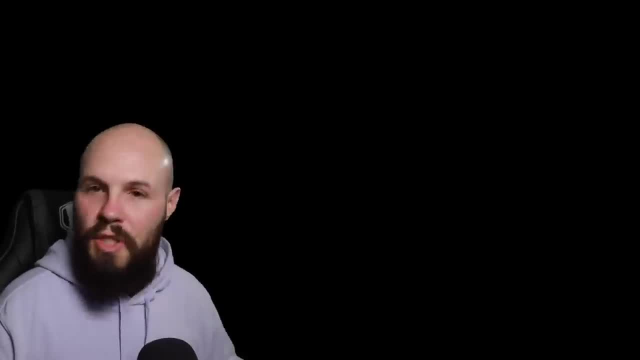 kind of copy that data and it's his own instance When you create a new one. I understand that probably didn't make any sense. I have a good analogy that I've used that will hopefully clear it up for you. So think of a reference type, which again is a class, like a Google sheet that you're 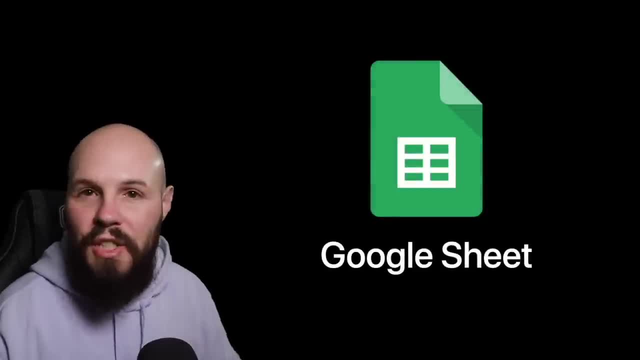 sharing with people. right, Like I create a Google sheet, I put my information in it and I share it with you. Now, if you change that sheet, you're also changing what I see as well. right, You're changing the initial source of truth. 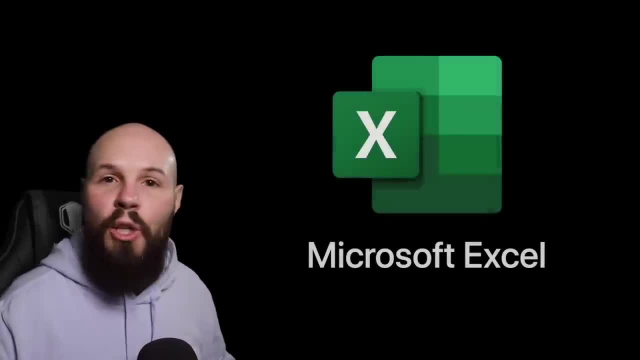 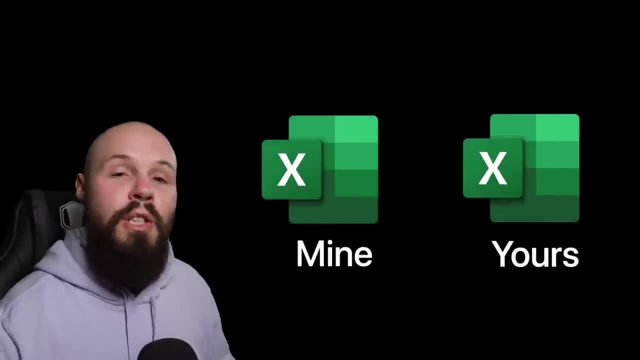 Whereas a value type or is like a struct is like if I were to create an Excel spreadsheet and then you know I would create it, I would save it and then I would email it to you like it's 2003, and then you would open up that Excel spreadsheet and use it as your own. 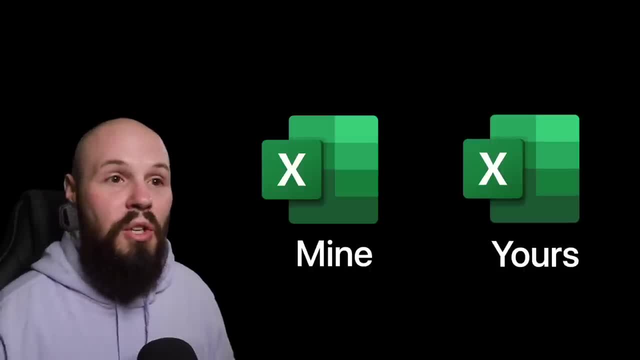 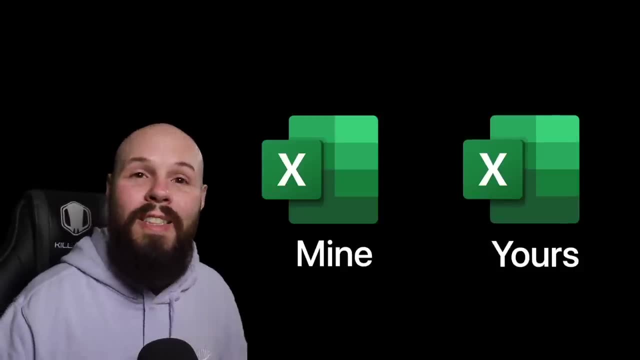 So the difference here is that on your Excel spreadsheet, no matter what you do to it, what kind of crazy changes You make, I still have my Excel spreadsheet. Like, your changes aren't affecting me, right? I made a copy of my spreadsheet, sent it to you and now it's your own thing. 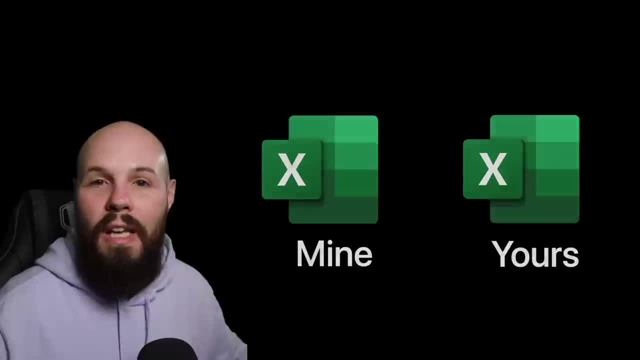 It's your own instance of your spreadsheet. Well, again, that is like structs and value types. Let's walk through some basic code to show you the difference. All right, so we're back here at our good old developer class and you can see, I've created. 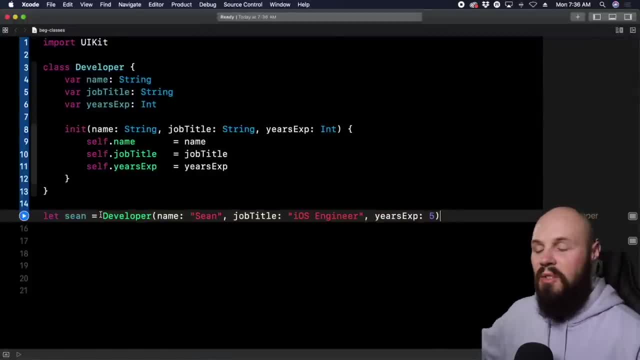 Sean. I've left that up there. So again, this is class, This is the reference type and I have Sean and let's change this to var, because we're going to be changing Sean around a bit. as you'll see here, Constant can't be changed. 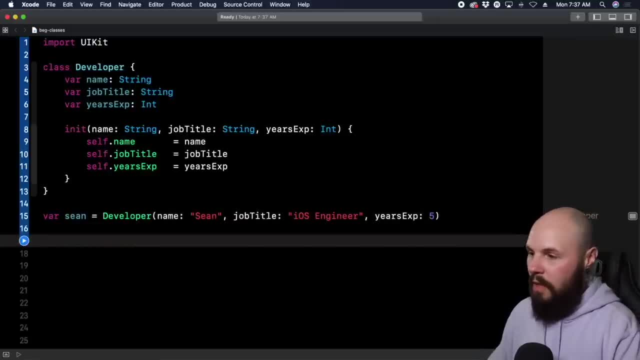 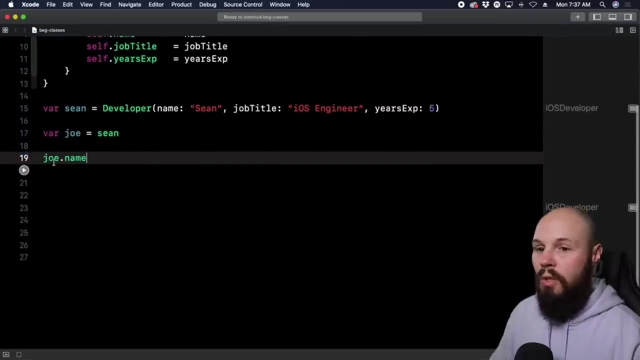 Var is a variable, can be changed, So I have Sean. Now let's say I want to do var. Joe equals Sean, So now Joe is still referencing Sean. So if I did joename and we'll scroll up a bit so you can see it and run it- 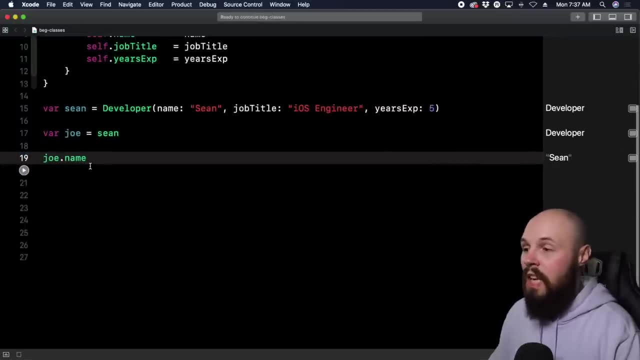 It's going to be Sean, because I'm referencing that. and then let's say I change this name, Say do joename equals, and then we say Joe. right, That would make sense. So we're going to run this. You see, now the name over here changes to Joe, as you can see. 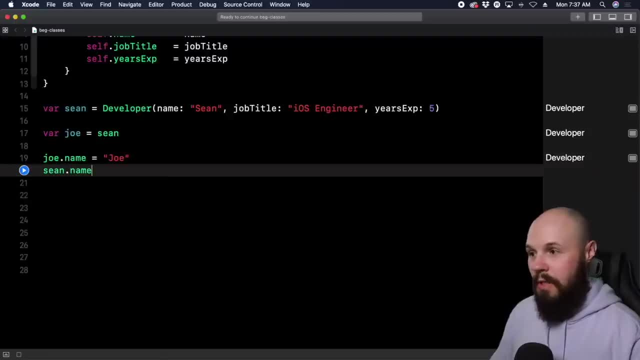 And now watch: when I do Seanname, it's going to be Joe. So run that Now. Seanname, as you can see, here is Joe. Just print it out right there, So Sean's name, even though I create or put it into a variable called Joe, and then I changed. 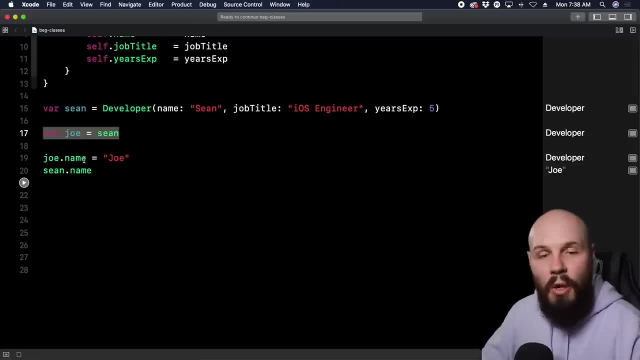 joename. Well, again, the reference all points to the same underlying data. So I changed Sean, even though I think I was changing Joe. So right, So Seanname now equals Joe, So that is a reference type or a class. Again, you're pointing to the same underlying data. 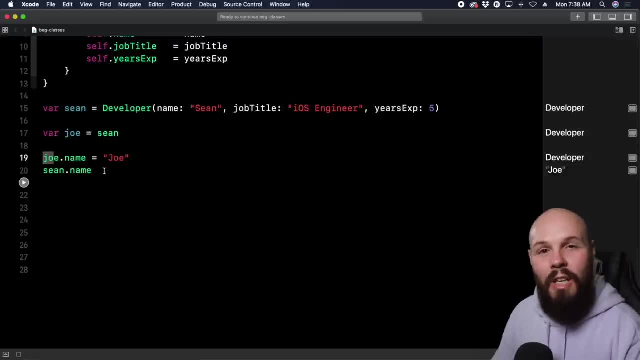 It's the equivalent of it being a Google Sheet. Any changes you make are all going to change the same source of truth, that is, reference types. So now let's talk about value types here. So scroll up to the top. Very simple: We just change this to a struct. 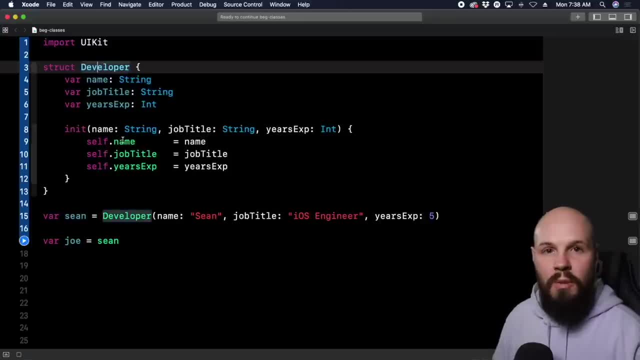 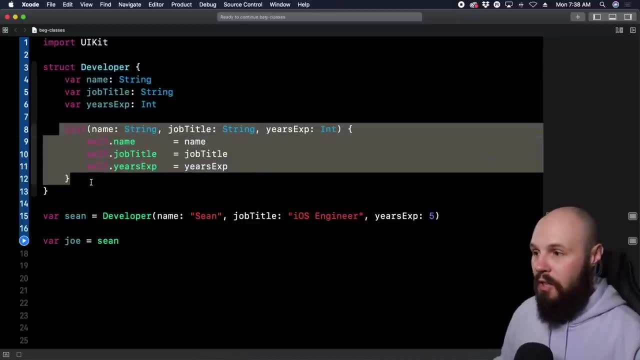 So now, this is a value type. One interesting thing with structs, though- and this is another kind of benefit- is you get what's called a member wise initializer. So, with a class, we had to create our initializer here, so I can actually get rid of this. 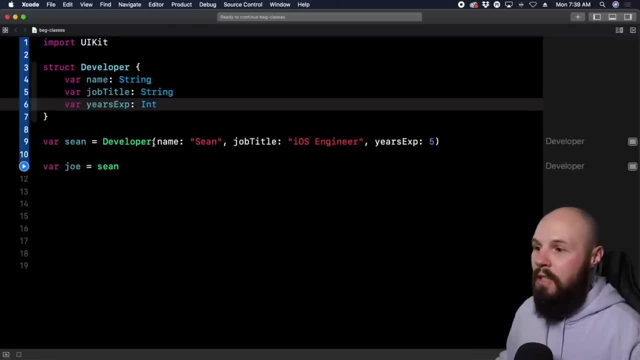 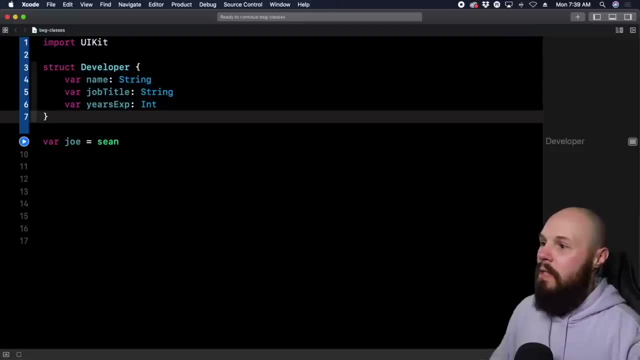 And Xcode and Swift are smart enough to know that it's going to give me this initializer, quote, unquote, for free, which is called a member wise initializer. Here I'm going to prove it So, if I can do: var, Sean equals developer, which is now a struct, and you see, I get this. 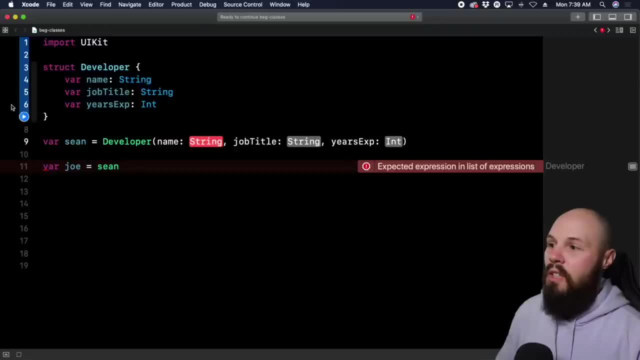 was called a member wise initializer for free, because it knows that hey put all these into an initializer, All right, so let's, I'm just going to command Z back to the to to get the type there. OK, so now we have our developer named Sean, which is now a struct. 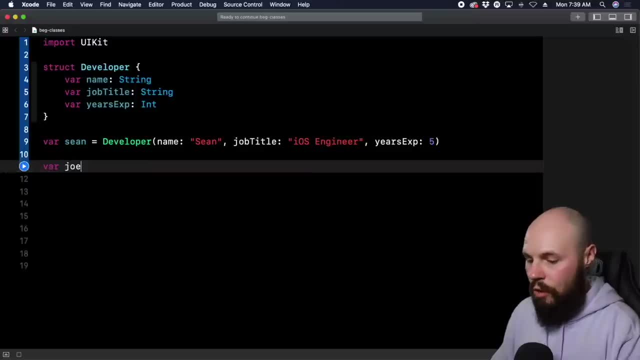 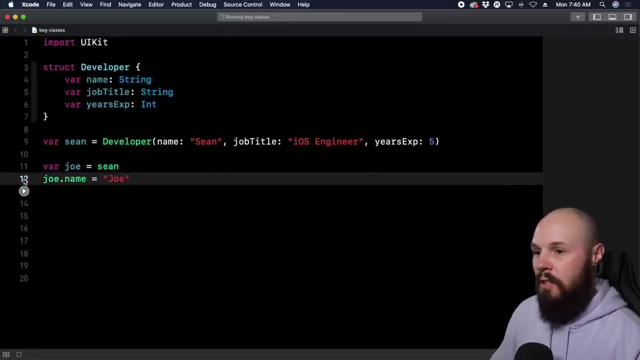 So now we're creating copies here. So let's do: var: Joe equals Sean. Now what this did is this: just basically made a copy of Sean and assigned it to Joe. So if I do Joe dot name equals Joe and I run it, we're going to get what we expect here. 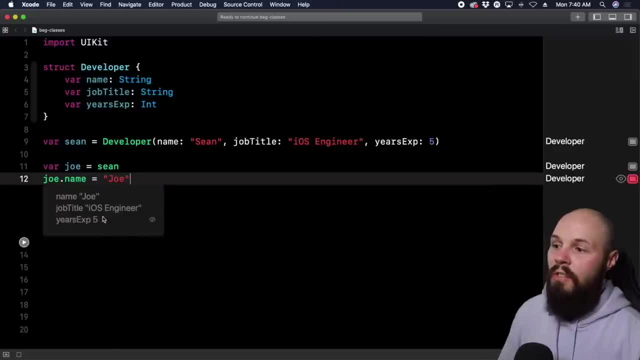 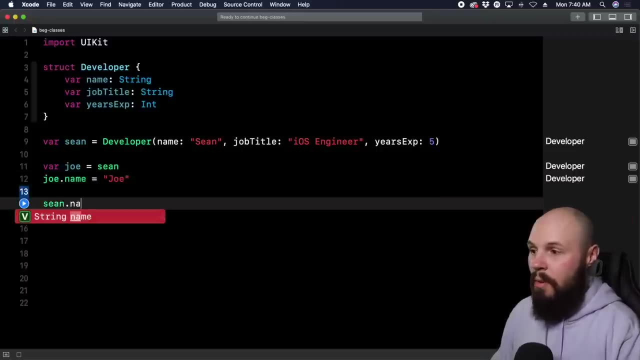 Joe's name, As you can see, is going to be Joe iOS engineer. five years experience again. we expect that we change Joe. However, Sean's name is not going to change, So Sean dot name. Remember last time it changed it to Joe because we did a reference type. 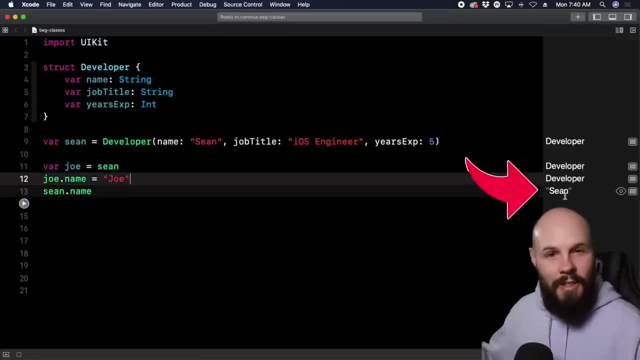 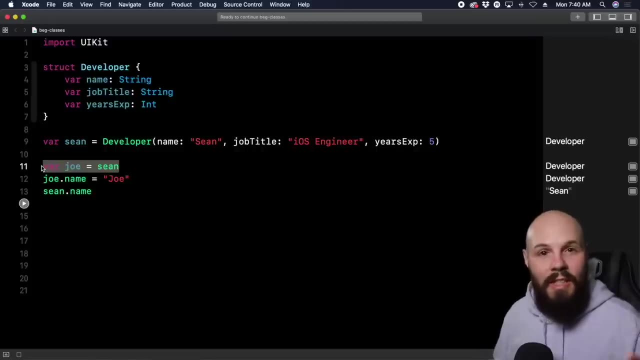 Well, Sean dot name is still Sean again, just like the Excel spreadsheet example. When I created this Joe variable here of a developer, I basically created a copy of Sean and assigned it to Joe, But I did not do anything to the original Sean variable up here, whereas, again, the 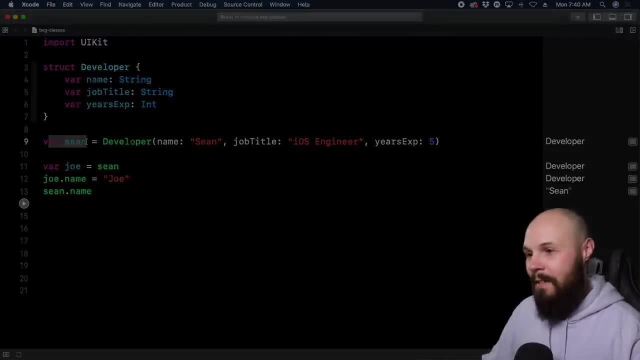 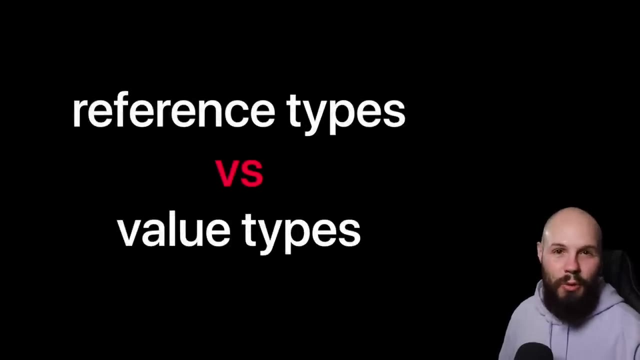 reference type. It was all pointing to the same data. We were changing that, So hopefully now you have an understanding of reference type versus value type. This is actually one of the most common job interview questions for your first iOS developer job. So if you're not quite sure you didn't quite follow again, hit up the comments. hit up. 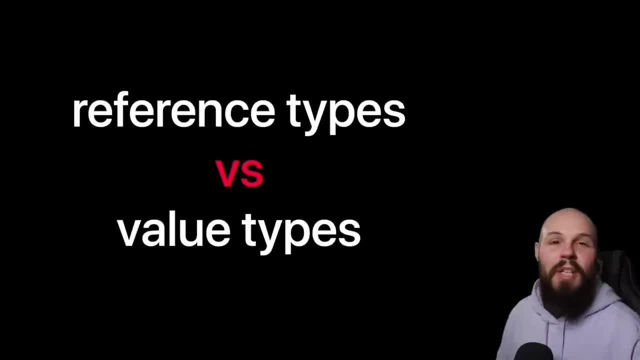 the Slack channel. Happy to help, But this is a hundred percent. You're going to get asked this in a job interview. If you decide to go that route, you can't avoid it again. Reference type versus value type- Key knowledge. 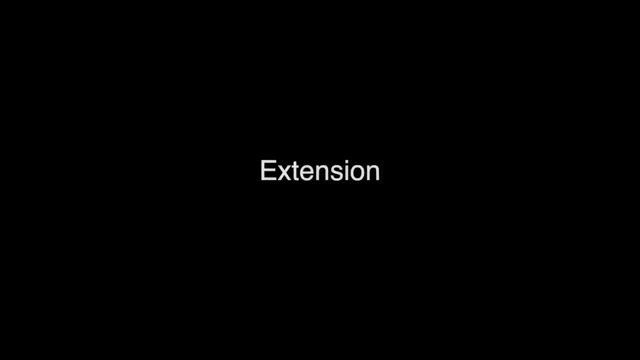 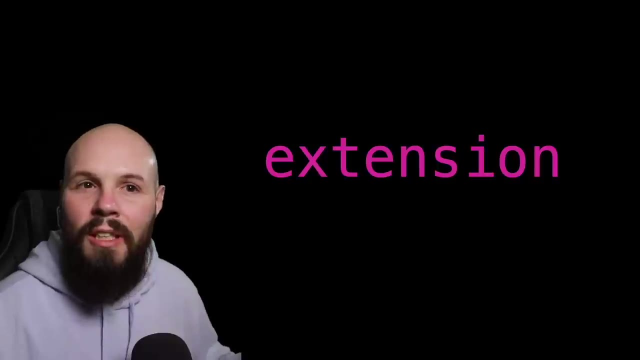 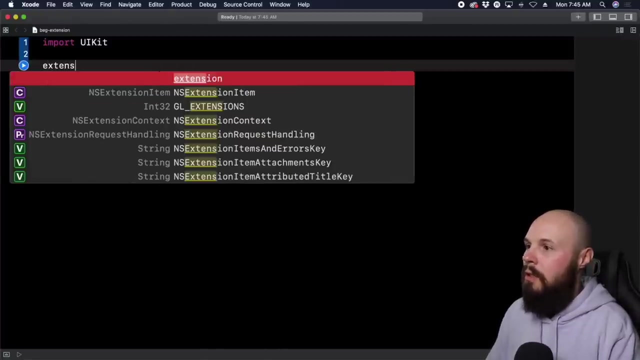 Hope you learned it Up. next let's talk about extensions real quick. So an extension is really cool. It's a way to add, like custom functionality to an existing type. Let's do a string one, for example, here, So we can do extension string and now we can give the string our own little functionality. 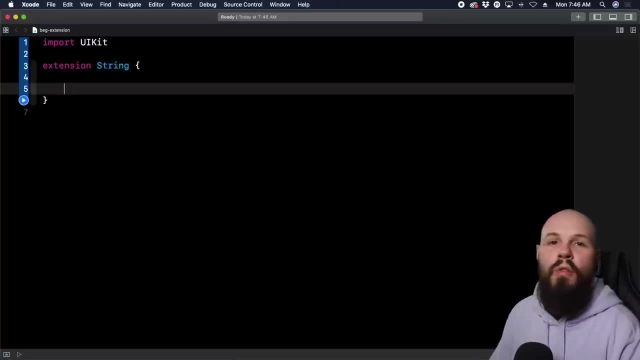 here. A common example that I've used in quite a few project is to remove the white spaces in between a string. So, funk, remove white space, Okay, And that will return a string, because what we're doing here is we're we're calling this. 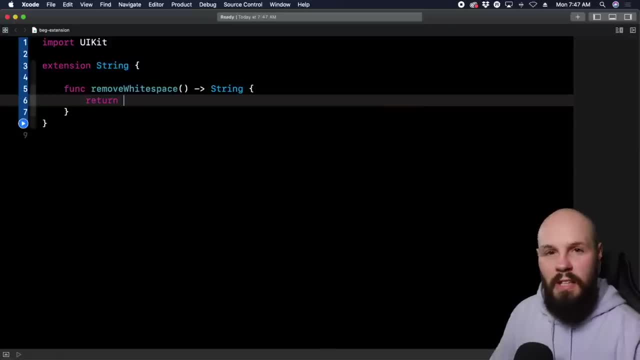 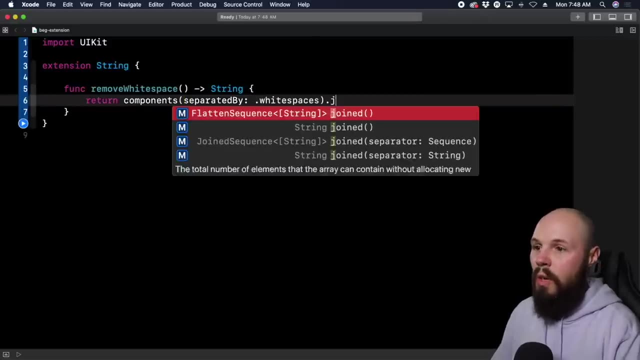 on a string, as you'll see, and we're kind of mutating it and spitting out a new string So we can return components separated by that white spaces and then we can do dot joined to bring them all together. So let's see this in action here. 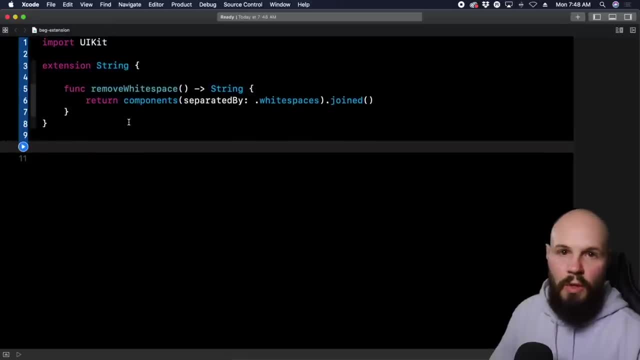 Don't worry if you didn't understand that code. That's just the example I'm using. Here's where, like the lesson is right here, Let alpha bet equal. I'm not gonna do the whole alphabet, But say you had A space B, space C, space D, space E, space F, Right? 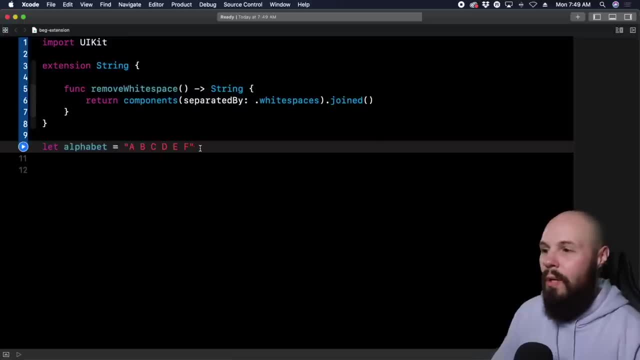 And you, you've got this string and you're like: no, I want, I want them all together, Right, I don't, I don't want them all spaced out, So right, We'll do this real quick. just to show print alphabet: run it. 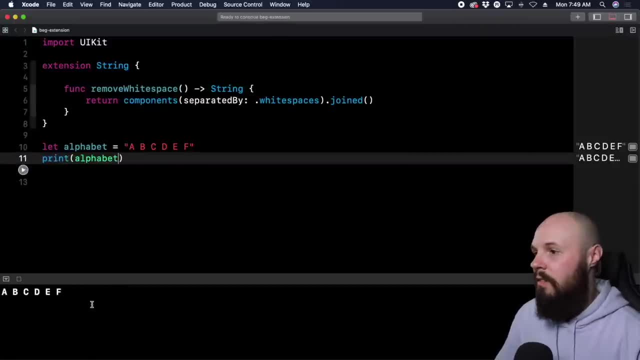 You're going to see down here in the console, right, It's all spaced out A, B, C, D, E, F. Well, if you did print alphabet dot, remove white space, which is what we just created up here on our string. 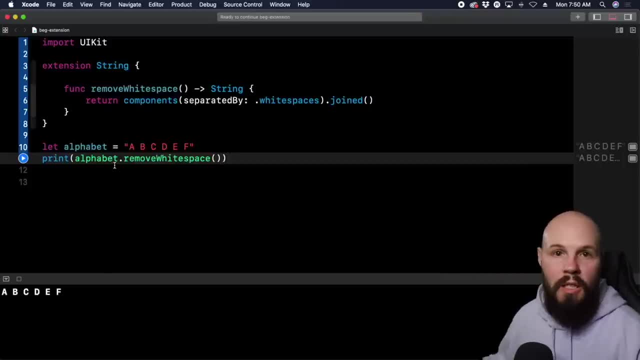 So by giving you this extra functionality, We can do our string dot and then whatever our new functionality is. So we did our string alphabet dot- remove white space- And now when I run it, uh, they're all no spaces in between, as you can see down there. 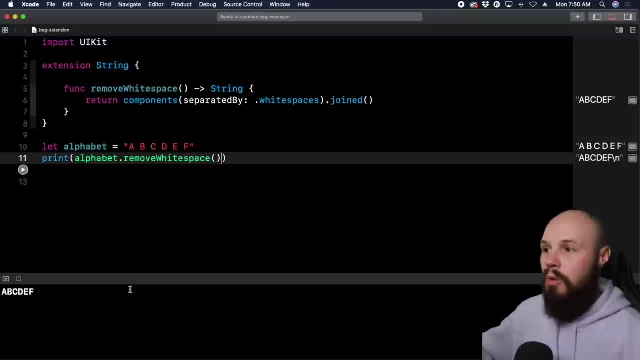 So again, the extension- and you can do this on ints, floats, bulls, doubles, whatever extra functionality you want to give. you can create an extension for it and give it that functionality. So it's a nice way to customize the types to your needs in your app. 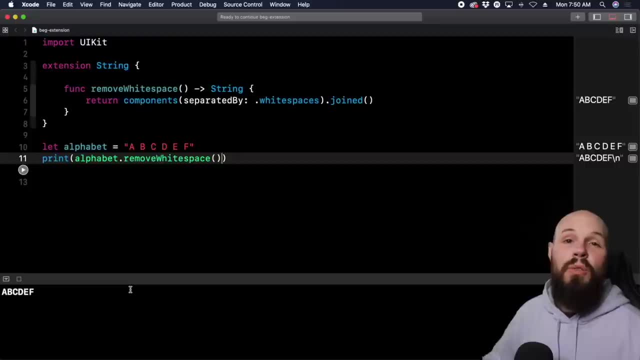 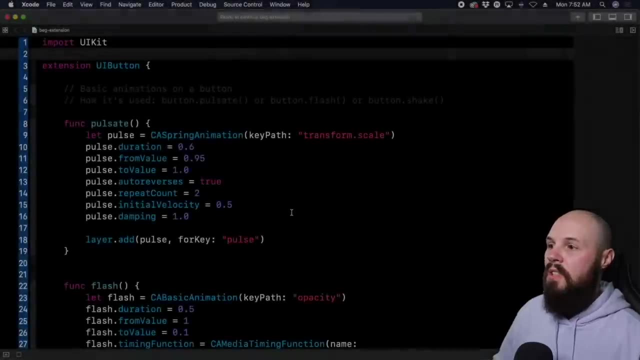 Now, one thing is this will give every single string the ability in your app To do this, which in this case is probably fine. but let's talk about a button example. So here in this example, we have an extension on UI button and you can see we have like. 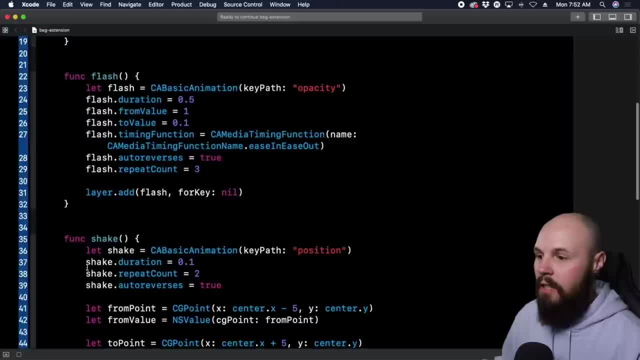 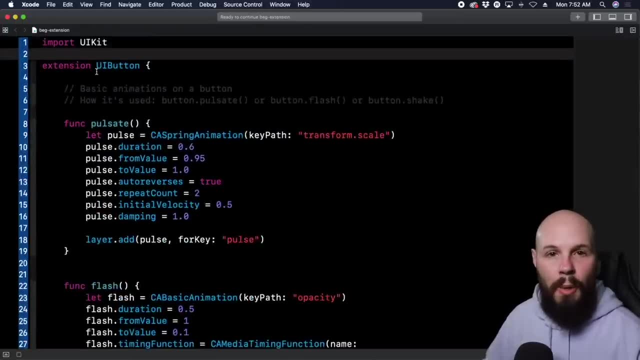 a pulsate and these are animations: pulsate flash shake. CB wrote out some nice animations, rounded corners. So again, this is the point I want to illustrate is that when you do an extension on a UI button, versus subclassing a UI button, which we talked about earlier. 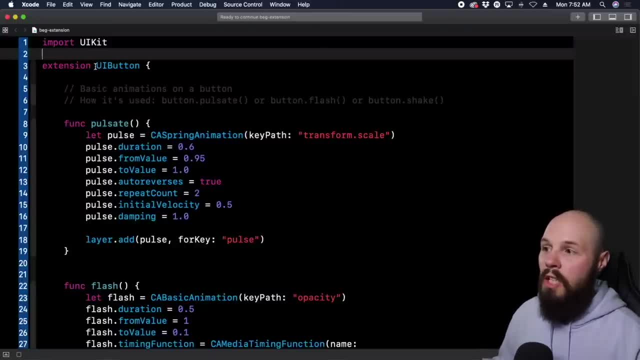 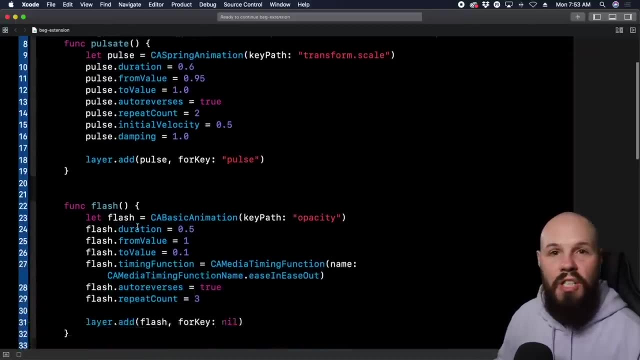 So the extension, like I mentioned, with the string, if I have this in my project and I do this in an extension, Yeah, It's going to give every single UI button this pulsate flash, all this functionality, every UI button. 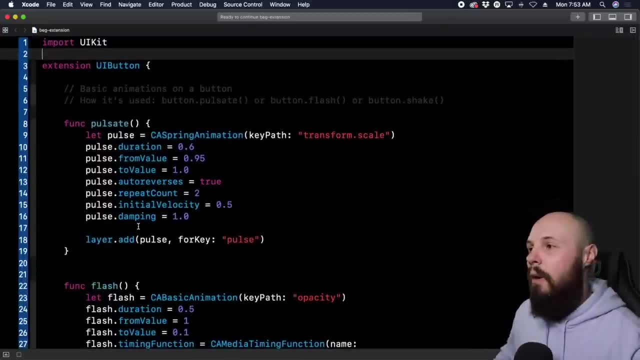 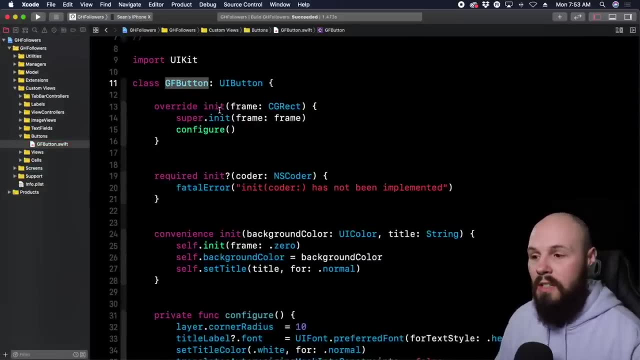 So that's what an extension does: It's pro, it's project wide, Whereas a subclass- if I go back to that example here- right, We have a subclass called GF button. So only this subclass is going to get this functionality right. 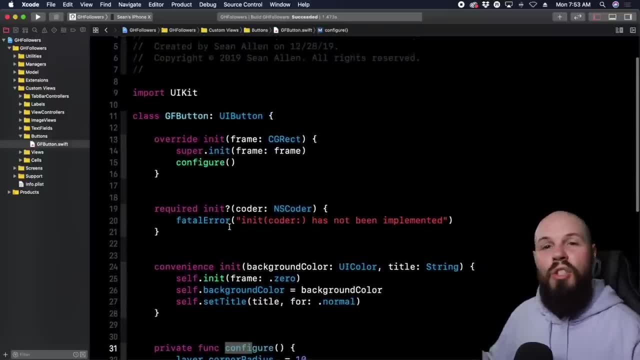 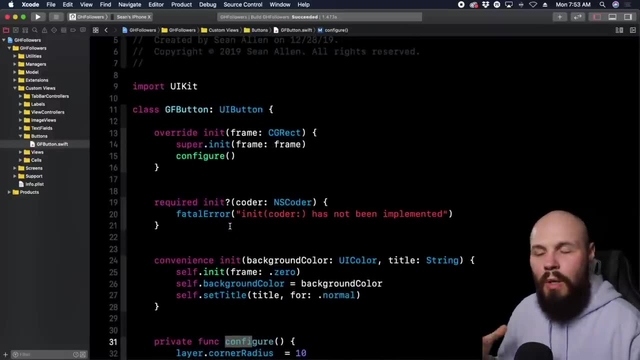 The configure the set background color. Now this is just one subclass of a UI button, but you can imagine in a, in a big app, you may have three or four different button types that you want to subclass. So when you subclass it, whatever functionality you give to those specific button types, like 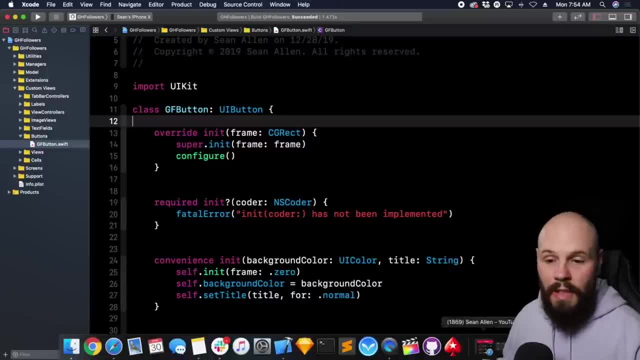 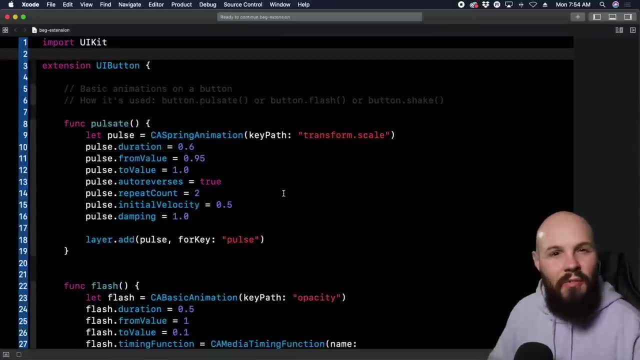 only they get it. However, the extension on the UI button- again back to this year, uh, gives it to every single button. So again, it's more. it's a matter of a granularity, like how specific you want to be with your. 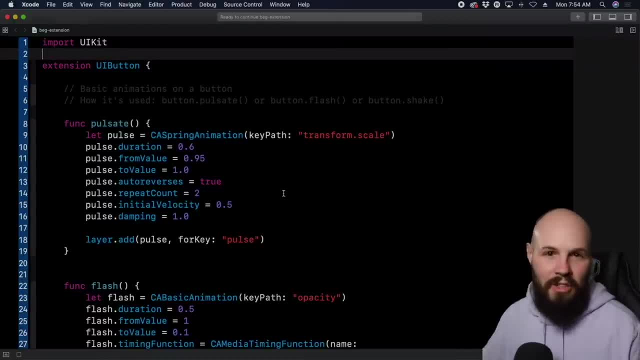 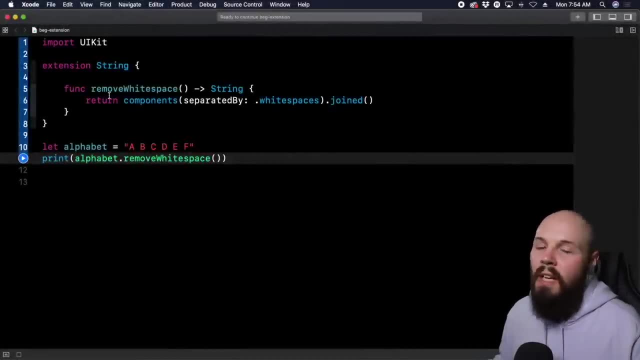 functionality, whether you subclass something or write an extension for it. So to reiterate back to our string extension again, we just added extra functionality to our string by removing the white space, And that's what you can do with extensions. Again, you can do them on classes. 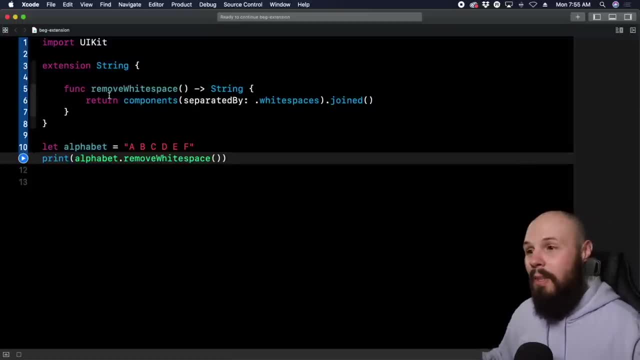 You can do them on types like ints, bool, string, um. it allows you to a lot of customization and they're pretty cool. I like them a lot. So, as always, if you have any questions, hit up the Slack or the comments. 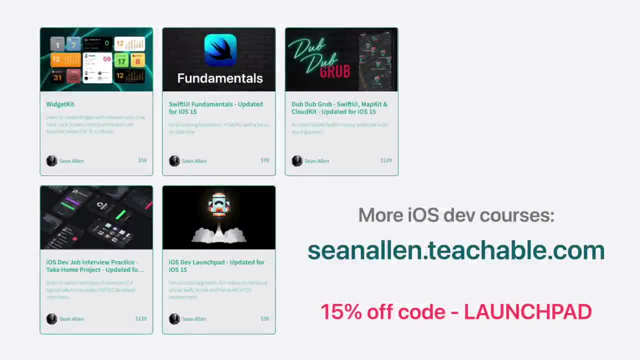 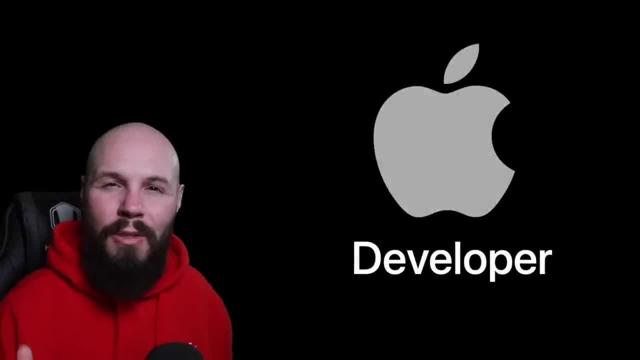 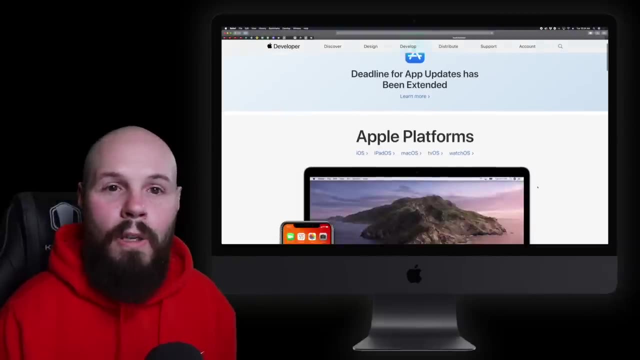 See you in the next video. What is the Apple developer program and do you need it? That's what we're going to dive into in this video. Here I am at developerapplecom. This is a website you will visit frequently throughout your career. 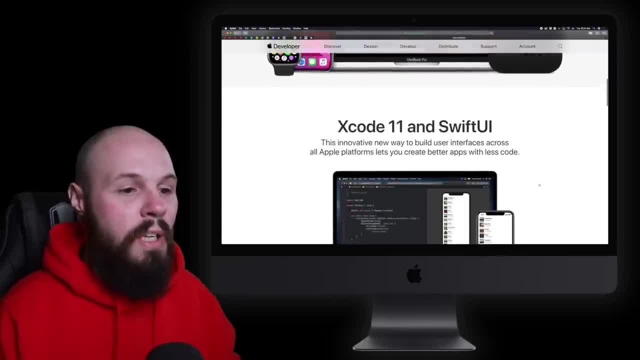 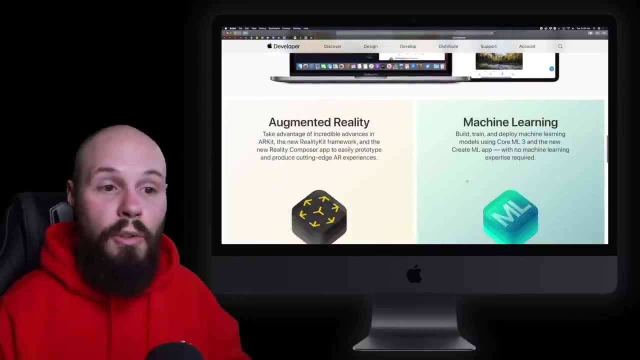 But I want to point it out in case you're not familiar with it. As you can see, you can get all kinds of information, uh about what's going on from a developer's perspective from Apple, like Swift, UI, Mac catalyst, the new frameworks, right. 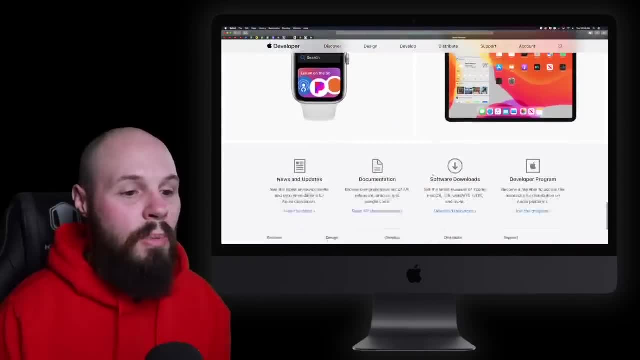 Augmented reality, machine learning. As you can see, I'm going to scroll down to the bottom here- Developer program. This is what we're going to talk about here, So I'm going to click on that and let's talk about what it is. 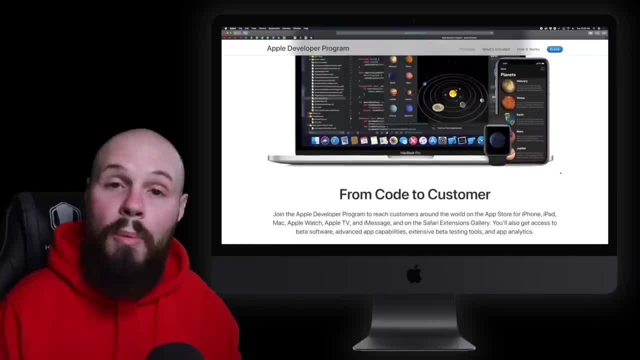 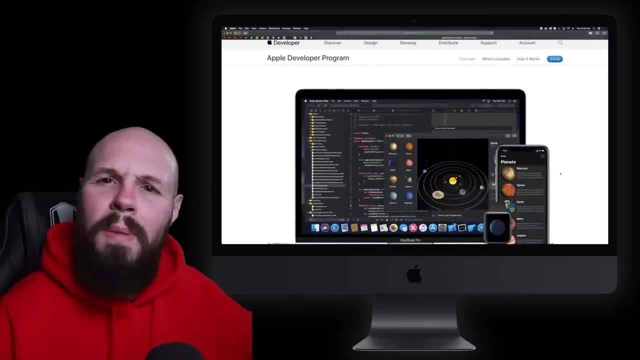 So essentially it's $99 a year. So it does come with a cost for you to be part of the Apple developer program. Let's talk about what you get for that And you know that'll lead into like: do you need to spend that money yet? 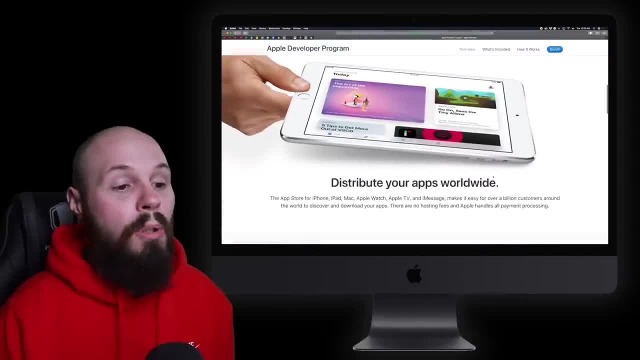 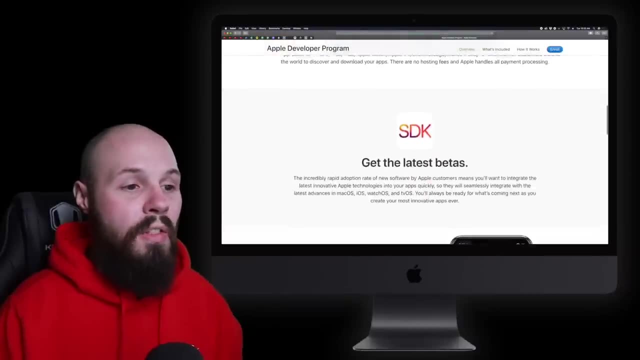 Um, so here, uh, you know you can publish your apps worldwide. So in order to publish an app on the app store, you have to have this developer account and keep scrolling. Uh, the latest SDK betas. uh, if you want access to all the betas that come out, so you. 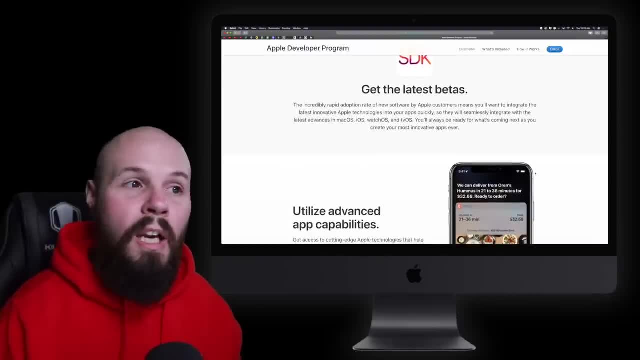 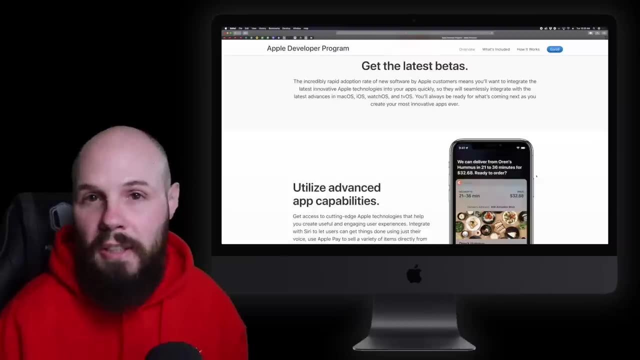 can work on the upcoming features before they're released to the public. uh, you'll need this developer account so you can download the betas, For example at WWDC. uh, they'll announce, you know, iOS 14 here in 2020.. 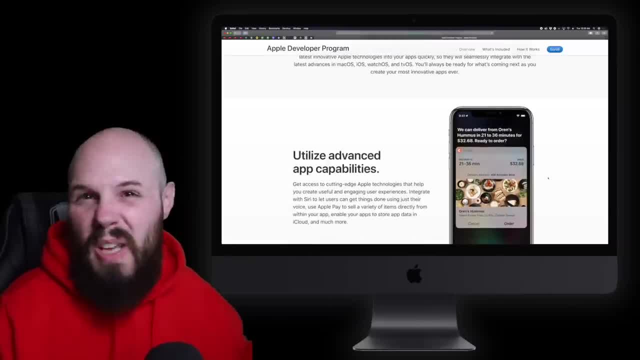 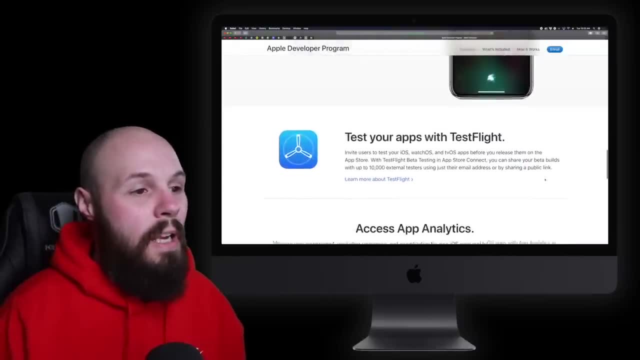 So you'll get access to iOS 14, you know, three ish months before the public does. that way, you can build all the new features into your apps, So it's ready by launch day. Um, and also test your apps with test flight. 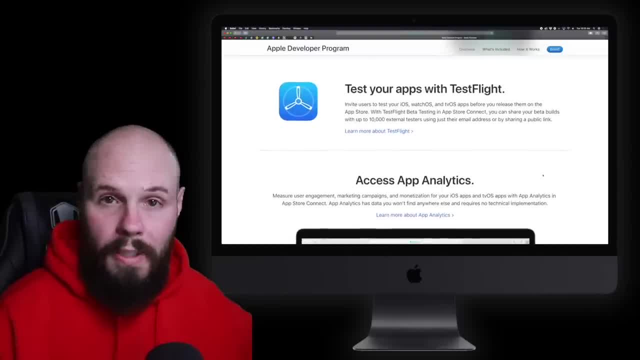 So test flight is Apple's program. They actually acquired it So you can beta test your app. As you can see, you can beta test it with up to 10,000 external users. So if you want to access the test flight, you got to have this developer account and then access to your apps analytics once you launch your app. So, basically, to answer the question is: do you want to test your app? Yeah, If you need to pay that $99 a year for this Apple developer account. well, the answer is hopefully eventually yes, but right now probably not. 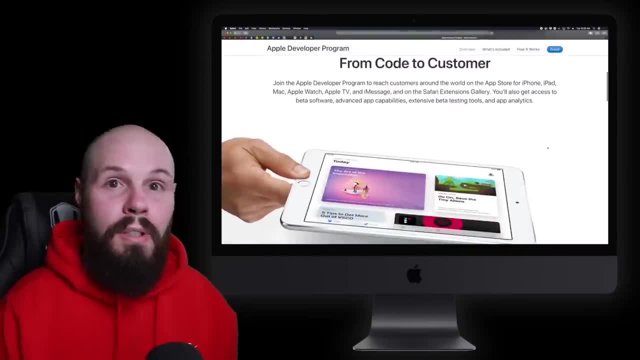 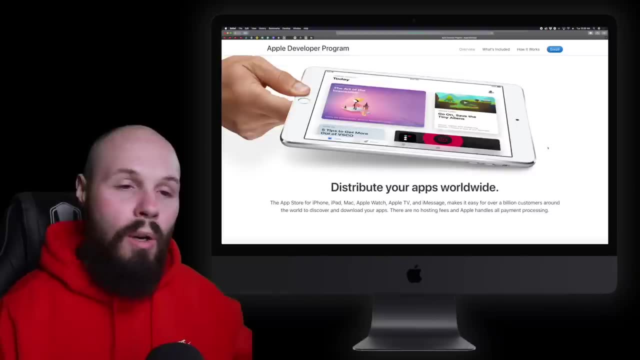 And why I say hopefully yes is because if you launch an app on the app store, you're going to have to have that account. Um, however, while you're building your app and just before you start beta testing, you know you can build it all without that account. 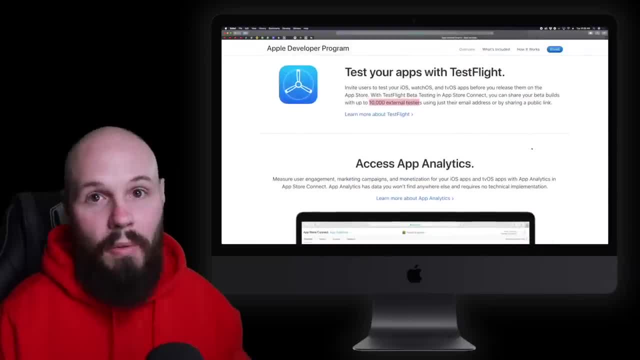 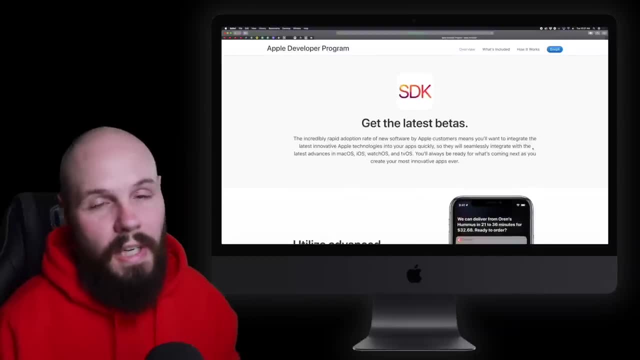 But again, when you're ready to put it on test flight, you're going to need the account. That's how you beta test your app. Uh, if you need to mess with With the new advanced SDKs, like the new betas, the upcoming features, you're going. 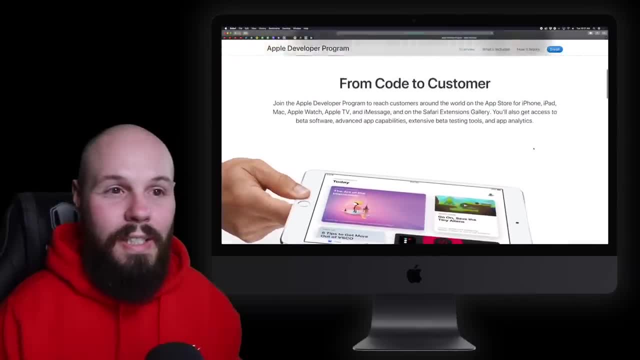 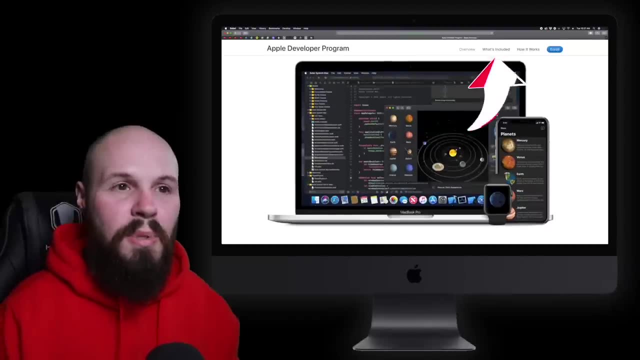 to have to have that account. Uh, so again, like I said, the answer is you probably don't need it right now, but hopefully you're going to need it eventually, And I'll link to this website in the description. Feel free to look around, but you see what's included. 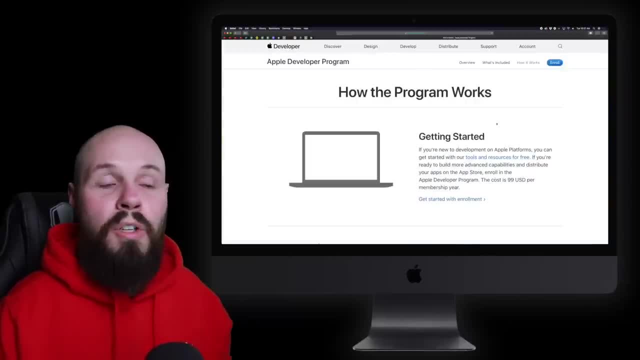 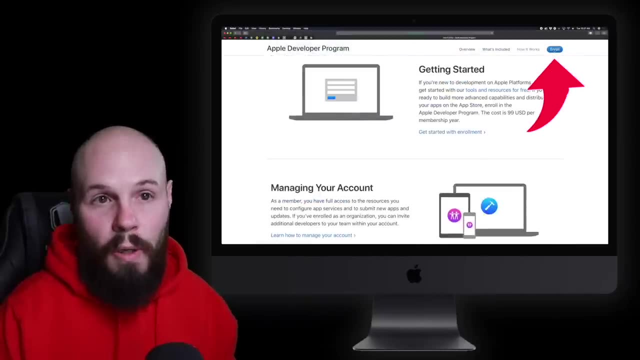 They list all kinds of you know stuff that you get here, how it works. they'll walk you through how to actually enroll into the program what it does, uh, et cetera. And you know obviously this enroll button right here. you can go ahead and enroll as. 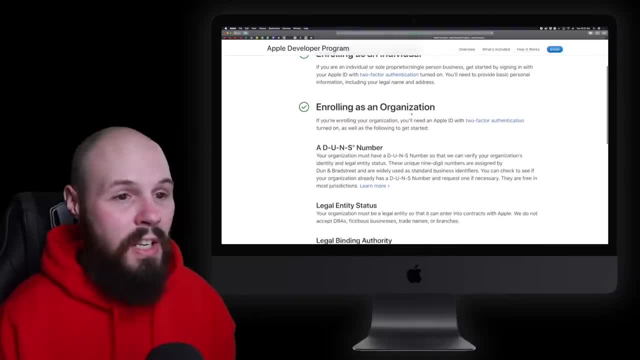 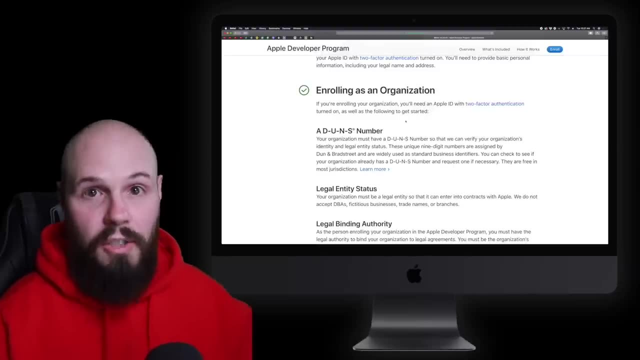 an individual or if you are like a company, uh, you can enroll as an organization. I believe the organization fee is a lot more. I think last I checked it was like 400 a year If you're enrolling as an organization, to where you can have multiple developers under. 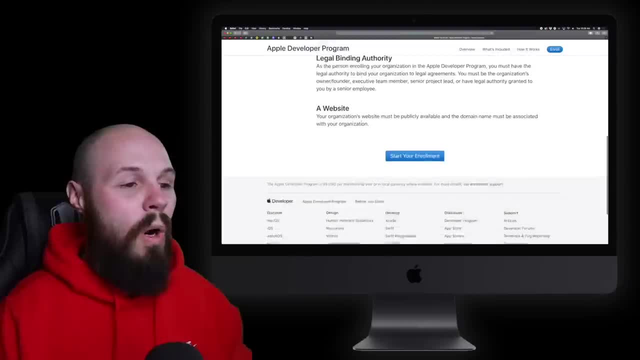 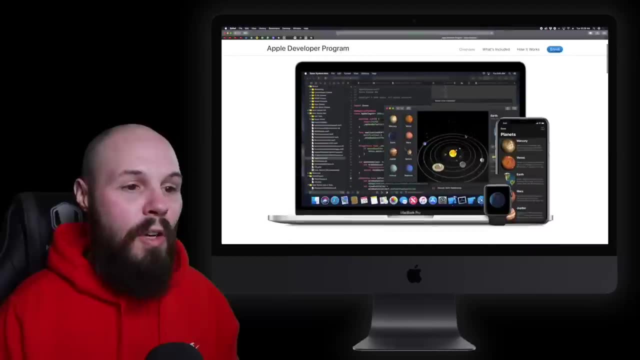 you. most likely you're going to enroll as an individual, Um, but again it'll walk you through the whole enrollment process. Again, start your enrollment. uh link will be in the description. but to reiterate, uh, apple developer program: $99 a year. 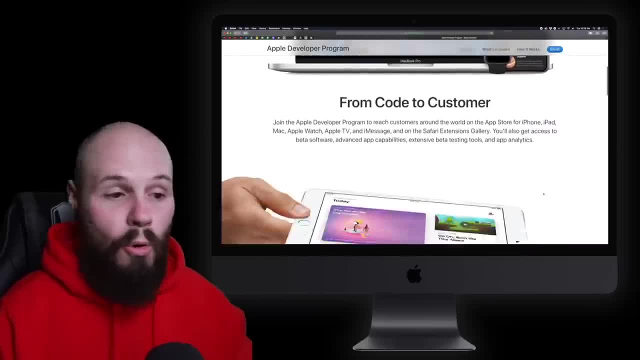 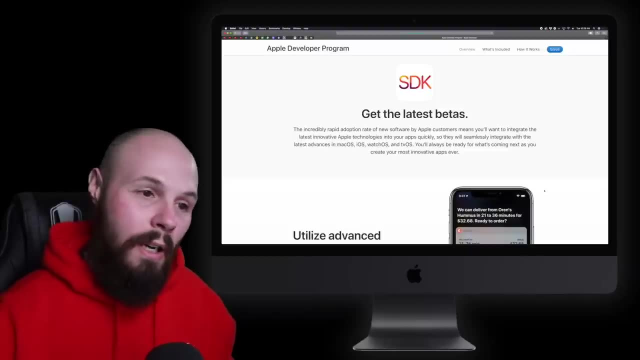 You probably don't need it right now, But if you're want to release an app or access the betas, Uh, you're going to have to fork over that $99 a year to apple. So if you have any questions about the developer program, uh, again. comments- Slack channel. 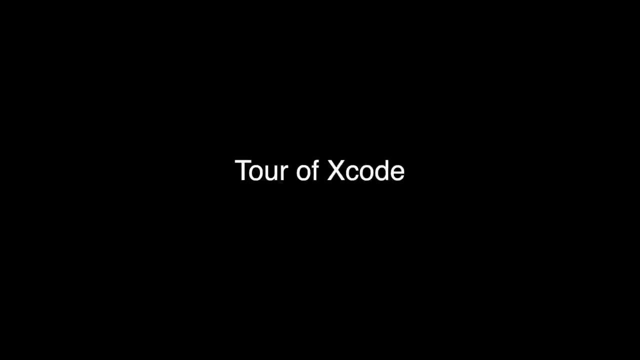 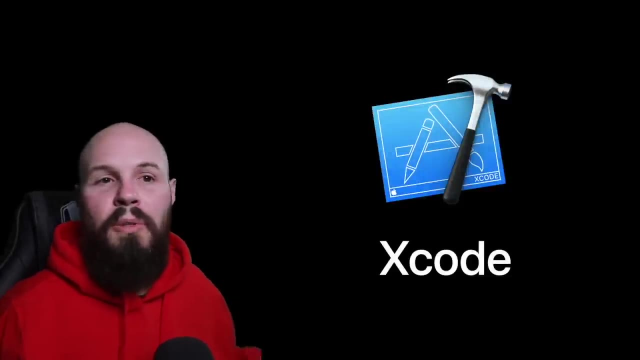 see in the next video. In this video, we'll be going through a very high level tour of Xcode. like the project, So far we've been using Xcode in playgrounds. Those are pretty simple. Uh, we're about to shift over into using Xcode for our projects, where we actually build apps. 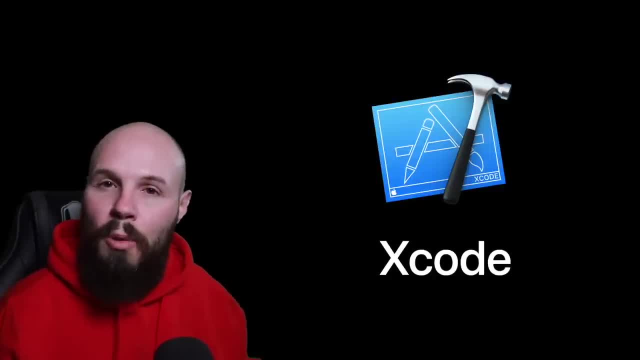 So before we do that, I want to give a high level tour Of the program, And this is just a super high level overview. uh one, because we're going to be using Xcode throughout the rest of the course, pretty much. 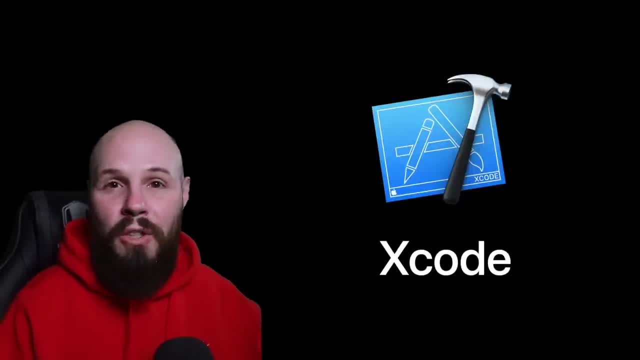 So you'll be picking stuff up along the way and I'll be pointing stuff out as we use it, rather than just data dumping everything up front. Uh, also, Xcode is a ridiculously huge program. I mean, ask developers who've been doing this five, 10 years. 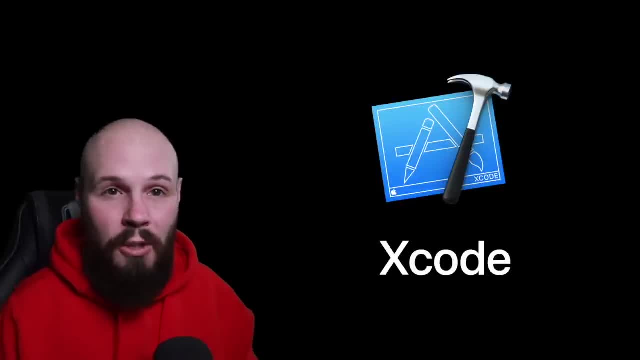 They're still constantly learning, uh, new things you can do in Xcode. It's just so big, Not to mention that it's constantly being updated with new features and new ways of doing things. Over a year, There are improvements, Don't get me wrong, but new things keep coming. 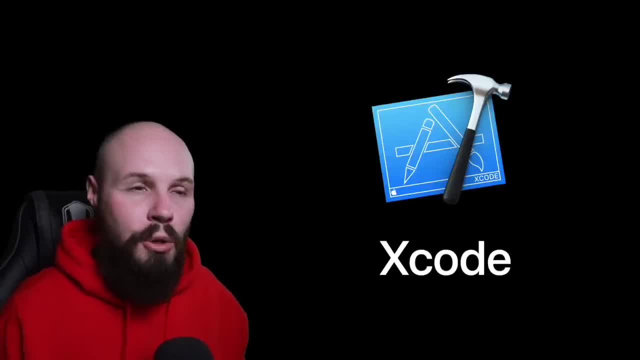 So don't be overwhelmed. Uh, Xcode is something you're going to learn and evolve with throughout your entire career. So, again, this video right here is just the super high level overview. The more you use it, uh- which we'll be doing throughout the rest of the course- the more 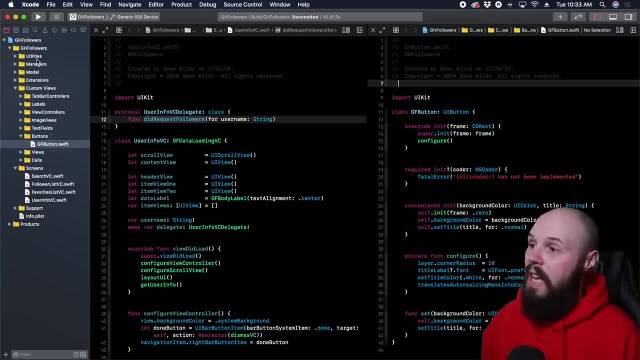 you'll learn it. So let's start off with this left pane over here that, as you can see, has our uh folder structures- Again the playgrounds. we didn't really have a folder structure where you can see my folders here. 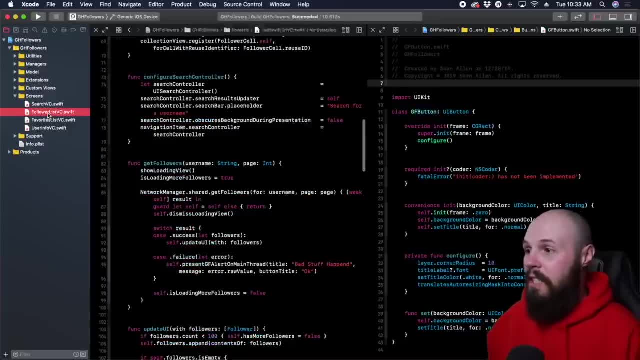 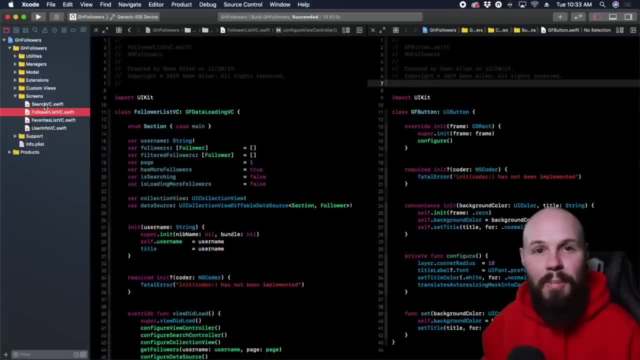 I have, like managers, models, custom views. Here are my screens and they each have the folders. you know that has the code in it. So, uh, file organization. uh, again, we'll work on this as we build our apps. I'll kind. 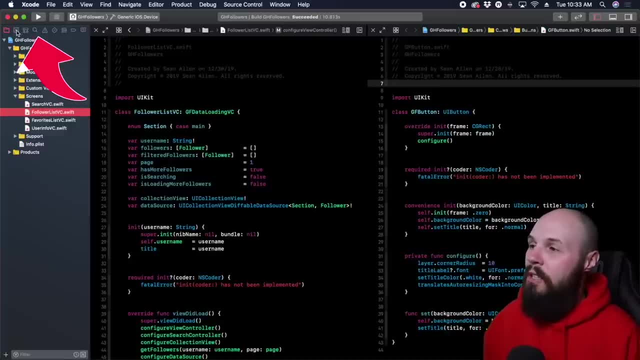 of show you how to do that. Um, but that holds this. but this left pane can do so much more. uh, up here in the top you can see there's a lot of options, like nine or 10 of them. The two most common ones by far that you're going to use are this: uh folder hierarchy. 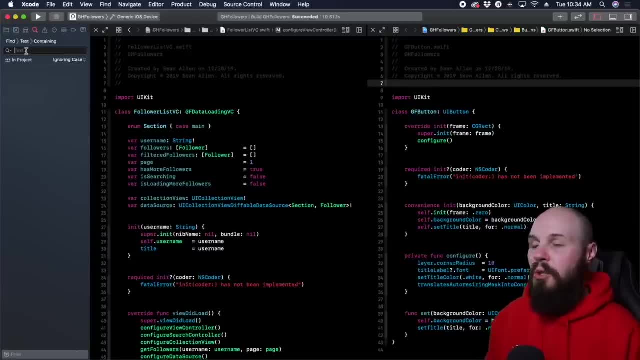 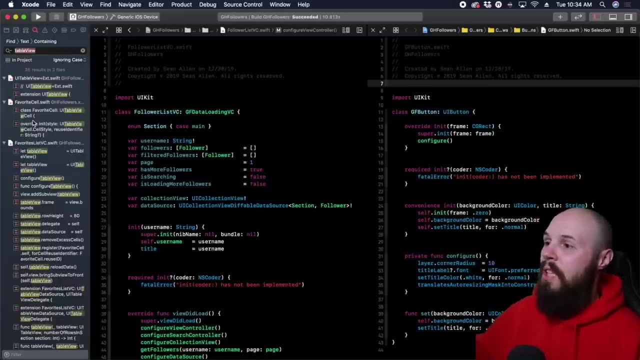 and then this search button, uh, or the search icon, here and here you can search your project. So, like you know, when did we use Table? if I spell it right, table view hit return. Anytime you use the table view you can see here. so it's a nice quick way to search your. 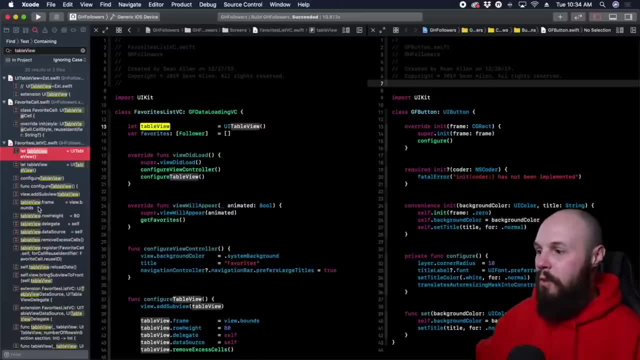 whole project and then if you click on it, boom, click on it, it'll take you right to that one. Let's say I want to go to this one. Oh, there we go. And then you see, all the table view sections are highlighted. 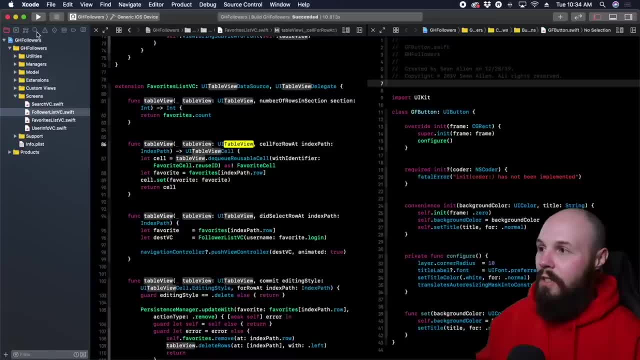 So again, the folder hierarchy on the left and then the search are by far the most you're going to use. You know this one will show all your errors and warnings, and then the rest are for like debugging and breakpoints. We'll get into breakpoints a little bit later. 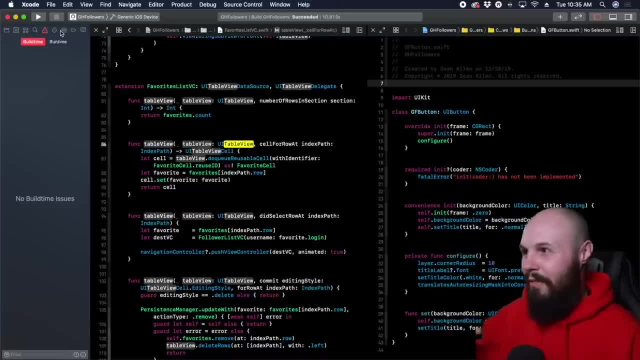 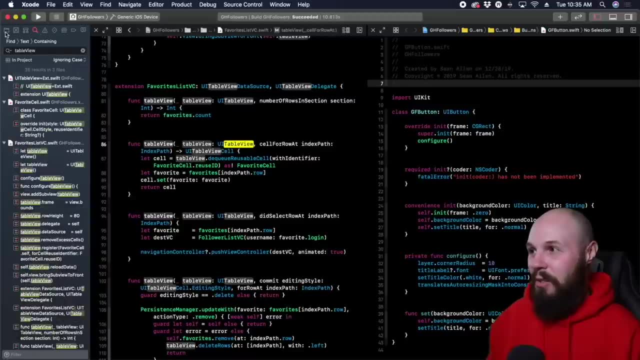 Um, Don't worry about a lot of this other stuff there for, like, advanced debugging, uh, source control, Uh, as a super beginner again, I would focus on the folder hierarchy and the searching. Those are the two that you're going to use the most. 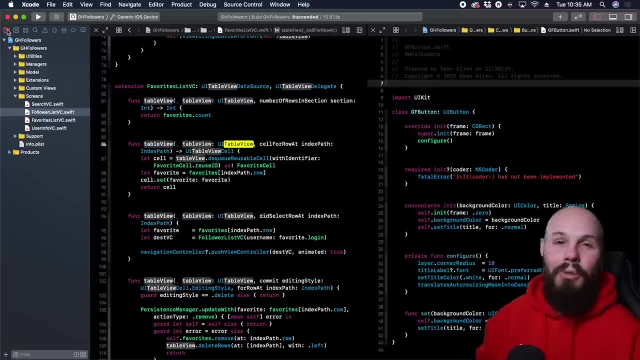 And again to reiterate, super high level overview. This program is huge. It's impossible to teach you everything And real quick. If some of you are working just on a small laptop screen and not a big desktop, you can make room here. 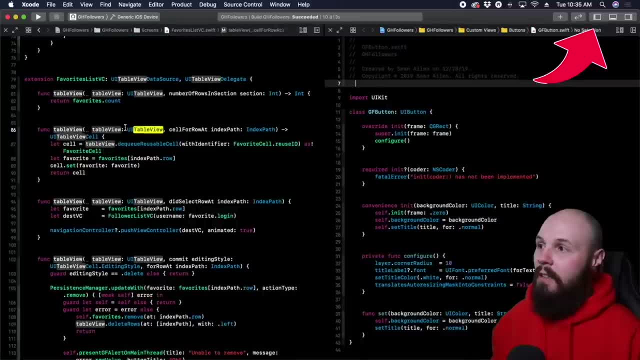 So here in the upper right, you see, the left pane is highlighted. Watch what happens when I click that: It hides it. Cool, Now I have a lot more room. Same thing with the right pane, which we'll get into. Uh, now I have a lot more room. 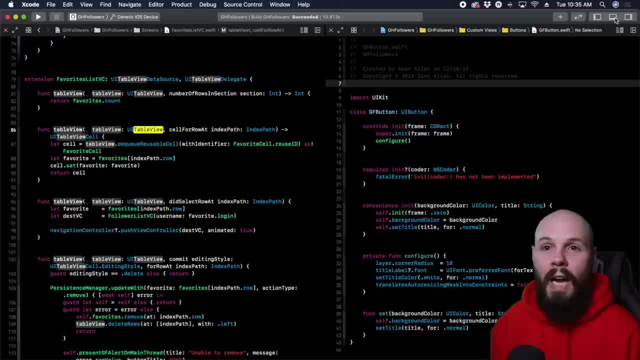 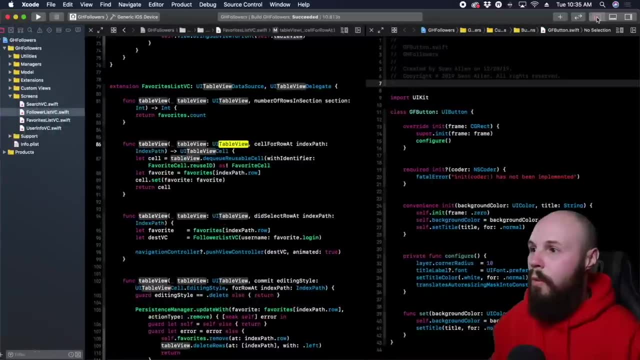 Uh, same thing. Your your debug console at the bottom. you can show and hide that. So if you need room on your laptop, there are ways to manipulate the UI so you can maximize your your room here. but we're going to bring back the left panel again. 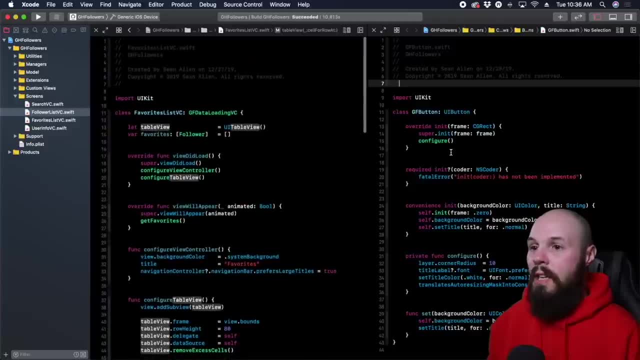 Now let's talk about the editor, which is what you see in the middle of the code here, right? So actually let me go back to the search, cause it's highlighting all my table view stuff, which is annoying me. Um, okay, there we go. 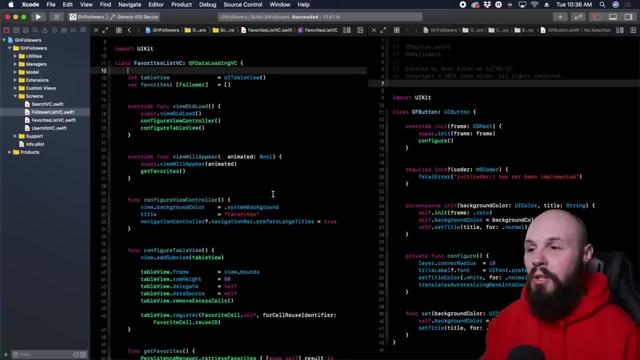 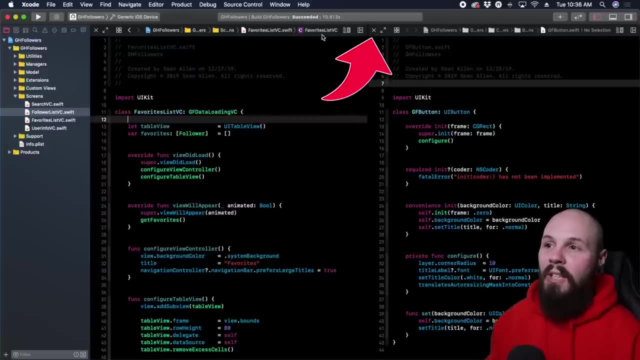 So back to the folders. So the editor- and this is how I usually work- I usually have two files side by side. Okay, Um, it's how I usually work, You don't have to. So here there's an X. you can see the editors are kind of separated, so you can close this. 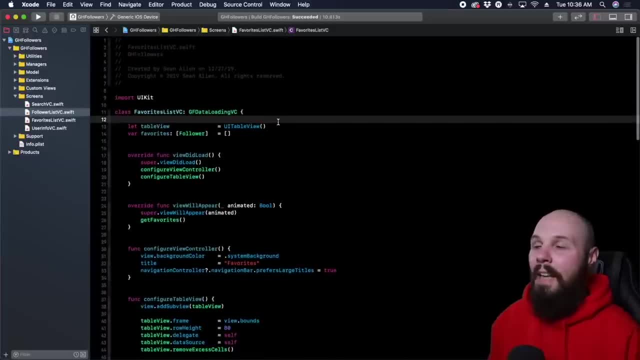 one out and just have one screen, uh, if you like. and the way to add another one is this little plus button. uh, right here that you see. So add an editor on the right, You see, you click on that. 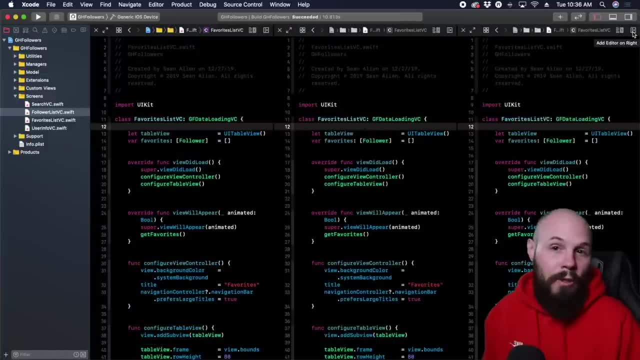 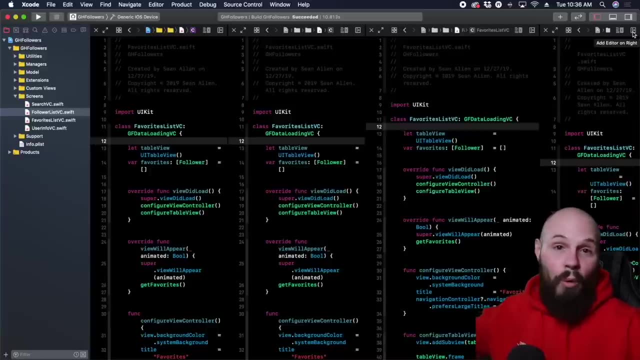 Boom, There's another editor. You know what you want to get: crazy. Let's add another one. How crazy do you want to get, I don't know. Let's add four. So if you had a ridiculous ultra wide monitor, uh, you could have four files, you know right. 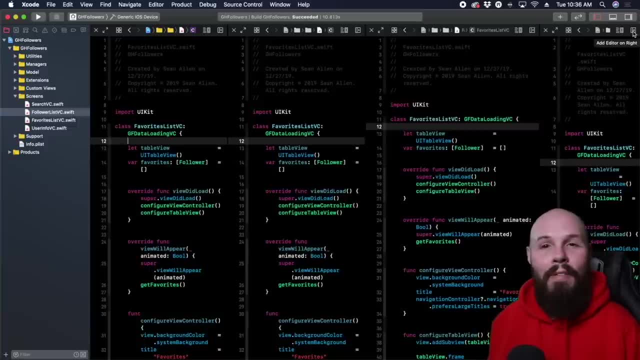 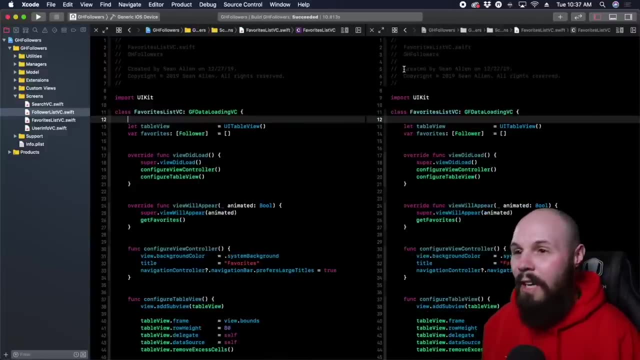 next to each other, And that would actually be a nice productivity boost. I can't say that I haven't done that And now. so let's close this out to make it not look ridiculous. Remember, I have my resolution on the screen blown up huge. 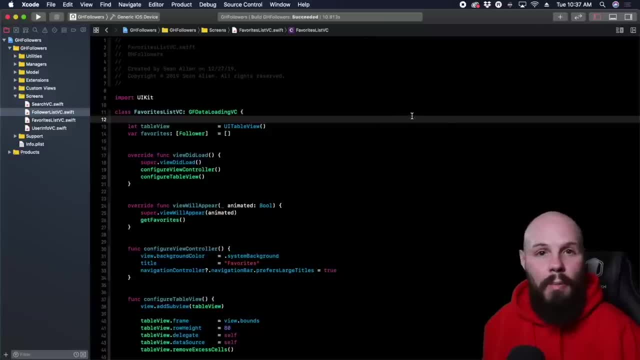 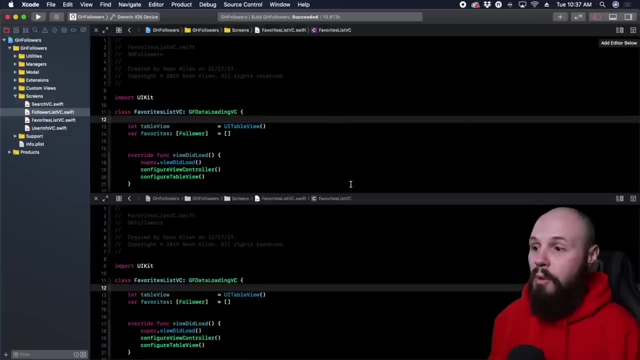 Um, so let's say you don't want it side by side. I don't know, Maybe you like to work vertically. If you hold option, watch this icon. you see the icon rotate so you can add an editor below. So you can go top and bottom if you want with your editors, uh, or side by side and uh. 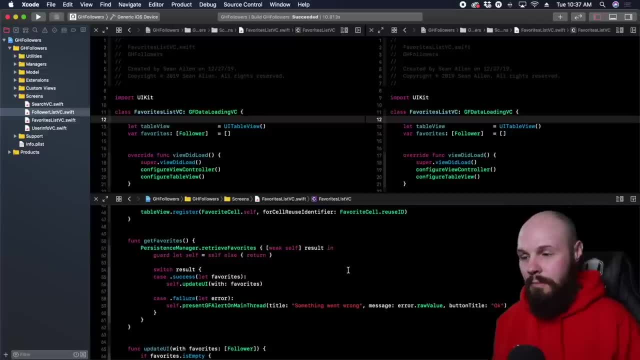 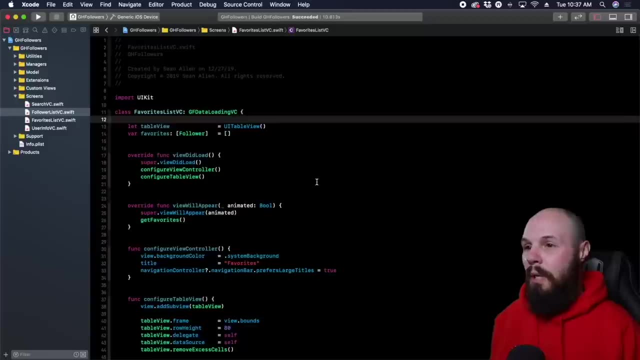 any, any mix of the two. right, You can have side by side, on the top Or on the bottom, So, uh, you can get real creative, uh, based on how you want to lay out your editors. But I want to show you that you can do that again, cause it matters, right. 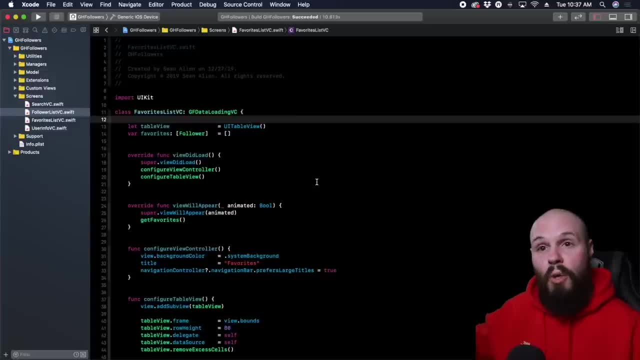 If you're on a small laptop screen, you may have one way of working versus if you're on a big external monitor, And I will point out, investing in an external monitor. If you are just working on a laptop, it doesn't have to be some crazy 4k ultra wide, expensive. 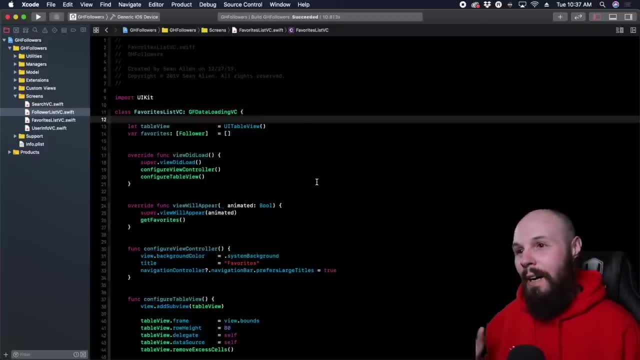 thing, but just the 27 inch monitor, Trust me. Uh, your productivity will go up. Life will be just so much better. It's I'm working on just a laptop when I'm working on a serious project, So something to consider. I'm not telling you to go out and spend all your money, but 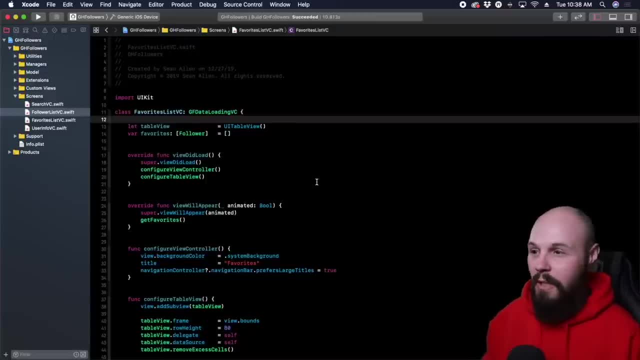 um, trust me you'll, it is a major relief to be working on a large monitor when working in Xcode. And also another thing that's fun here: the the icon to the left. here you can. there's some options you can do, uh, but we want to show the mini map. 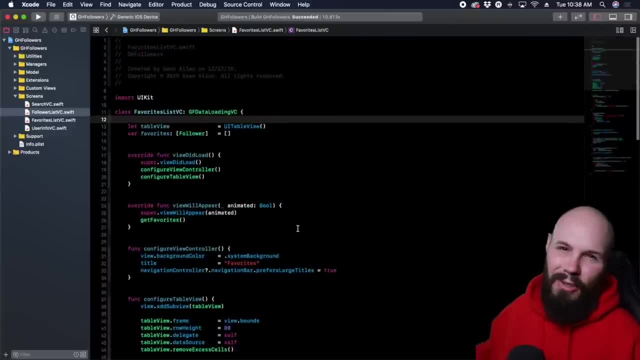 So this is a mini map of your code. So you have a super long file. None of my files are really super long, and but this will give you the mini map and you see, as I'm hovering my mouse over it, like it's showing me what function it is, as I highlight. 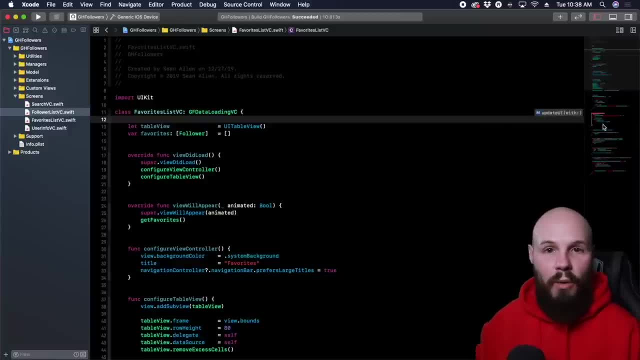 it, uh, and there's. There's other ways to organize your code: uh, so that it'll have breakpoints in the mini map. So if you do have a really long file- which, to be honest, you should try to avoid that- 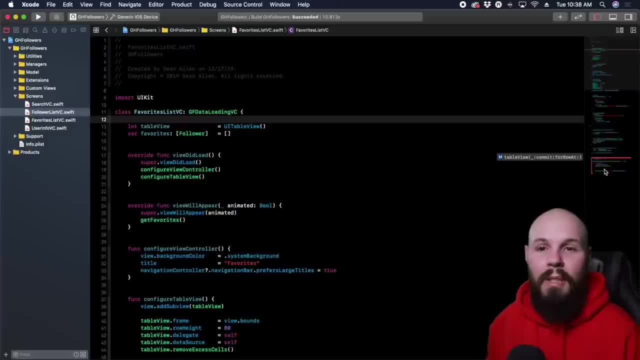 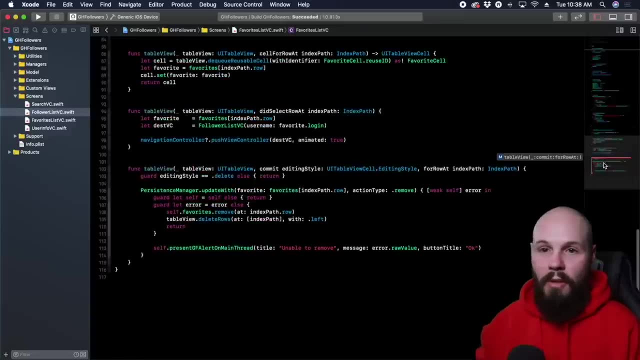 Like that's, if you have a thousand line file. that's not best practice, But for some reason if you do. uh, the mini map is a nice way to kind of navigate through that quickly. You watch when I click on this we go right down to the bottom. click on the top of the. 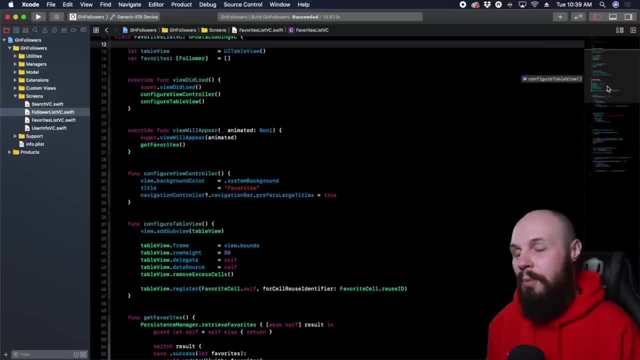 mini map and view to load right back to the top. Uh, so the mini map is a pretty cool. that was new in Xcode 11.. So pretty new addition there. Now let's talk about the simulator, like how you actually run your code. 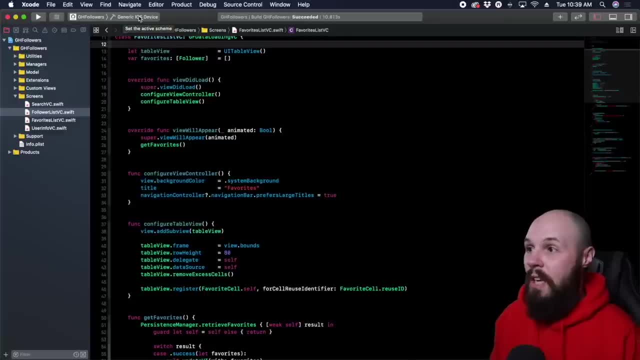 So up here, uh, in the upper left, you'll see I have a generic iOS device, cause I haven't selected a simulator where you can see I can choose iPhone 11, iPhone 11 pro, iPhone 11 pro max. I can run it on the iPad, uh, et cetera. 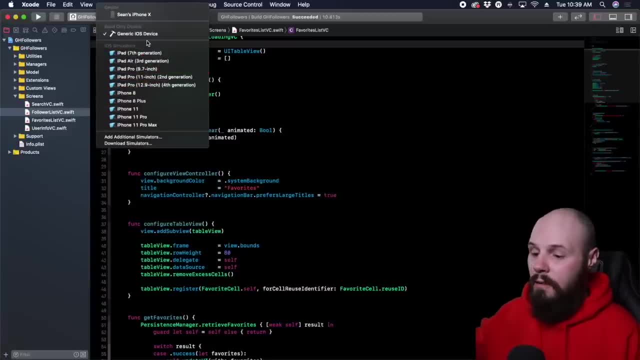 And, if I scroll up a little bit, I have my phone plugged in via a lightning cable. So now I have access to my phone that I can run the app actually on my device. We're going to do the simulator just so you can actually see it on the screen. 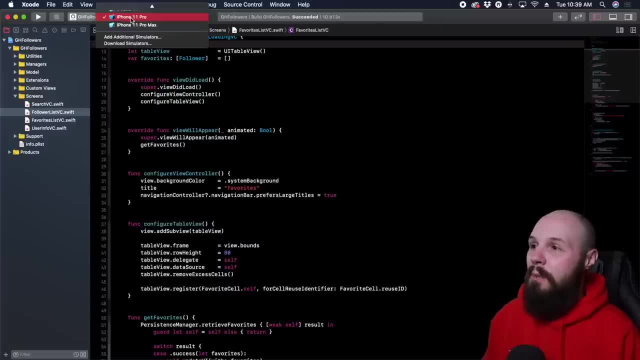 You can't see the screen of my device, Um, but now, once you select your simulator and you click on that, Whatever phone you want to run it on, if you're testing different screen sizes, uh, now you hit this play button and that runs your app. and you see, in the top, you'll see. 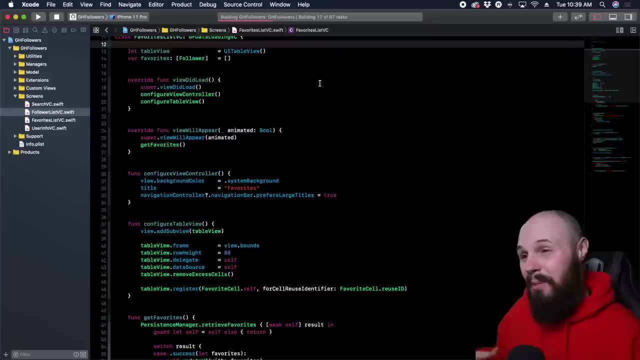 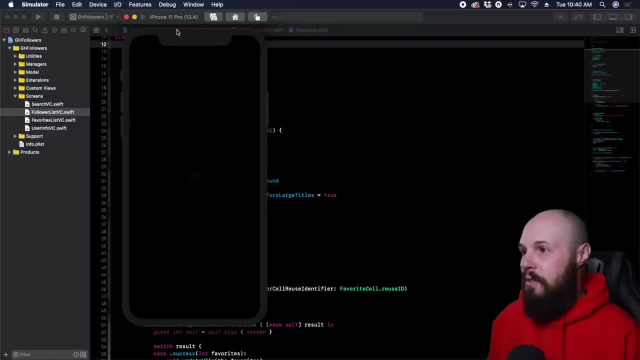 this progress bar. uh, depending on how big the app is, Sometimes this takes a really long time. Um, so, but anyway, the simulator we'll pull up here, uh, in a second. here you go. here's the simulator, as you can see, and it's going to run. the get a followers app, the, uh, my 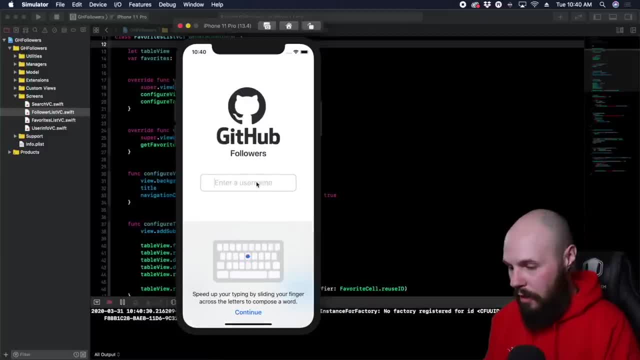 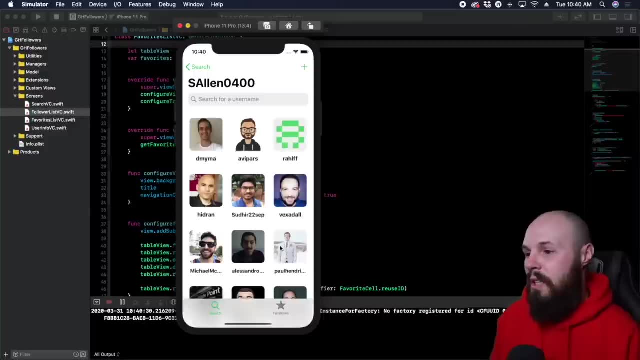 take home project course. So there we go. There's the simulator. Uh, you can use your app just like it was a an iPhone here. So S A L E N 0 4 0, 0.. Let's get my GitHub followers. pull those in. 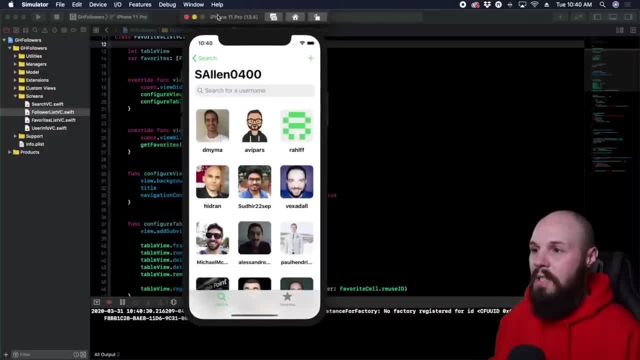 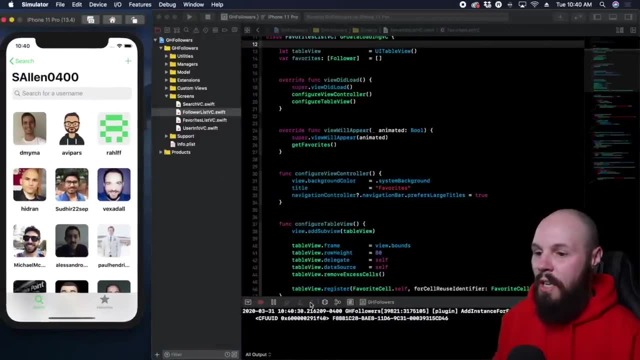 There you go, And the cool thing about the simulator is you can test various different environments. So let's actually, uh, move this over here so you can see the iPhone as I change it. Uh, this little button right here is called the environmental overrides. 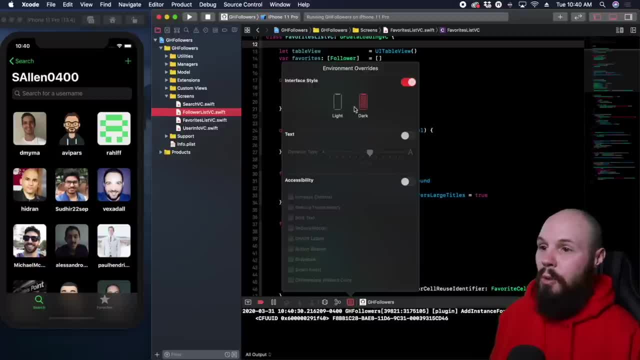 So if I want to go to, uh, we'll turn an interface style: boom, dark mode, click that light mode, dark mode, light mode. So if you want to test your, your app and light and dark mode, and if we go to, let's. 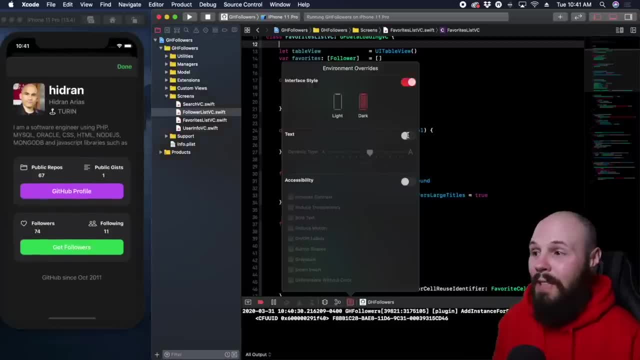 pick a follower, We're here. Uh, now you can also test your dynamic type So you can see uh. as we scroll you can see the type of our dynamic type. uh, based on the setting, is changing live on our simulator. 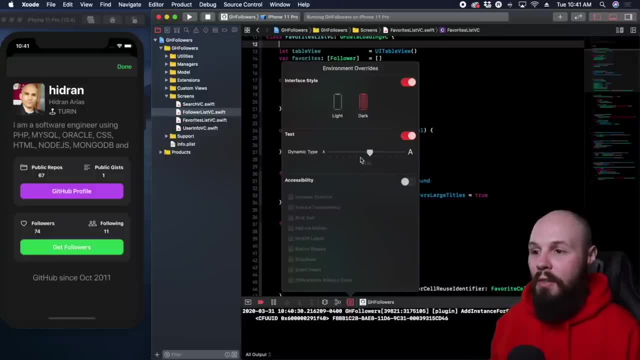 So this is a way for you to test various different aspects of your app and then all these options down here. I won't spend too much time going through this, but environmental overrides are a great way to test your app in various different- uh you know- environments, so to speak. 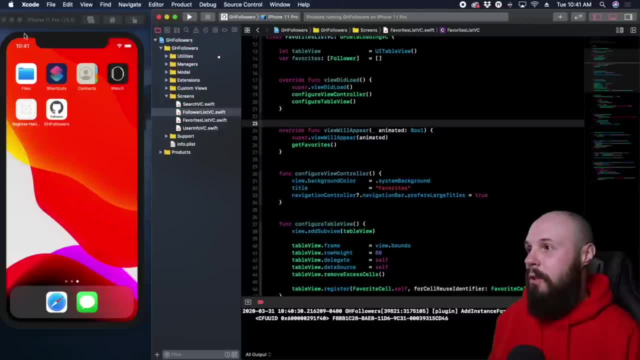 So, to stop your simulator, hit that stop button and then your simulator will be up. We're going to close it. We're pretty much done with that. Now I'm going to show you how to use a break point, which is a basic debugging. 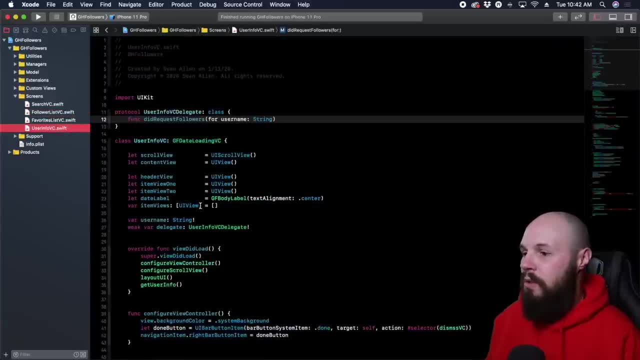 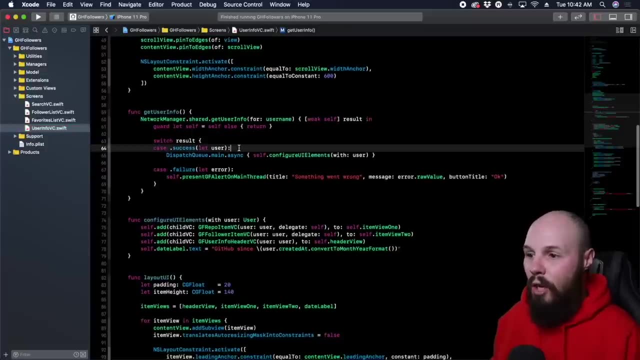 Let's get our debug console out of here. Let's go to our user info screen. Uh, basically the way this screen works is we pass in the user information and then we download that information from a server. So I'm going to put a break point just by clicking the line. just click on it left. 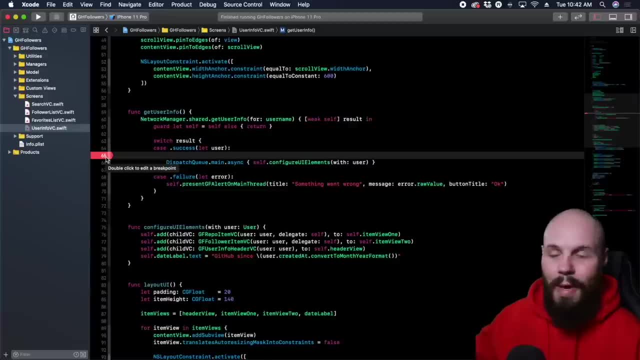 click on it, You'll see that red thing. Well, it may be a different color based on your, your max settings. Uh, maybe it's blue, but you'll. you'll click that there. That'll be a break point. 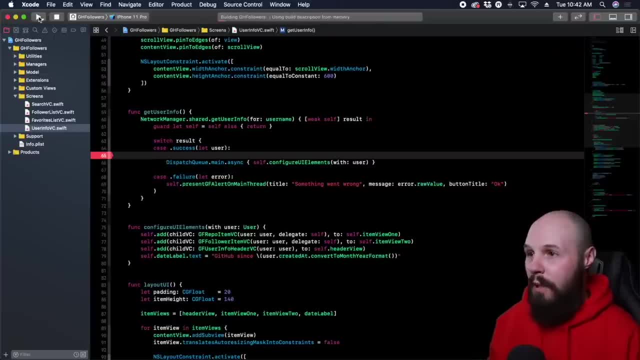 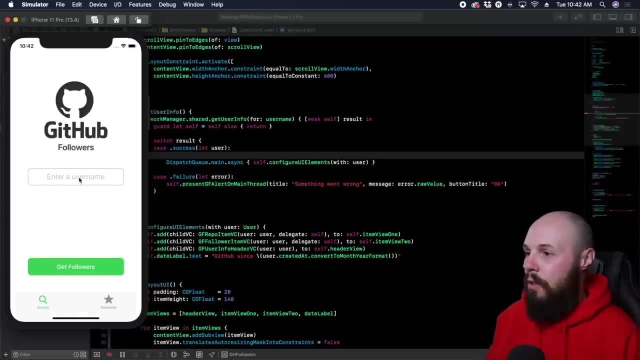 What that means is your code will stop executing. So let's actually run the app again and we'll get to the point where I'm trying to pull in the user, and then the code will stop executing and you can debug to see what's going on. 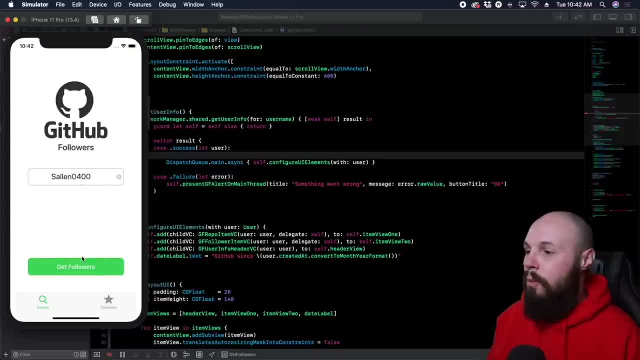 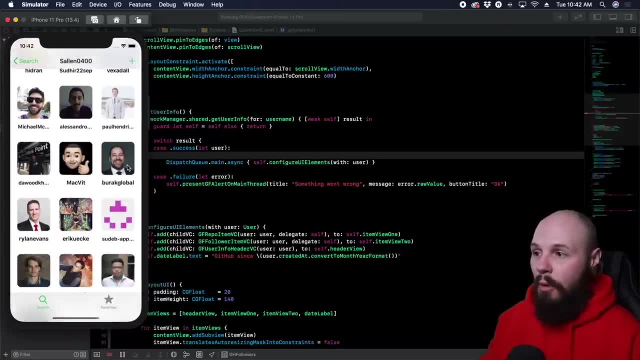 So here we go. Uh, we're not pulling in a single user yet We'll pull. we're pulling in all my followers. So when I click on a follower now, we're pulling in that user information, So the break point will stop. 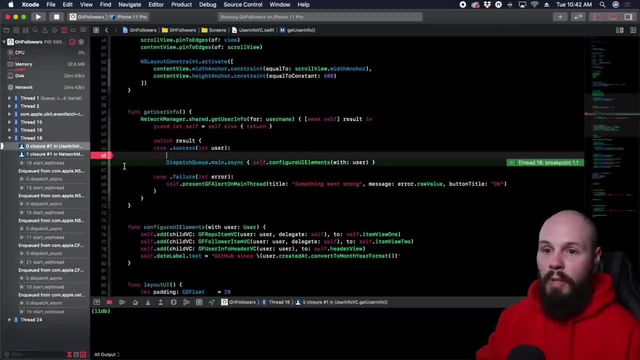 So watch what happens when I click this, I click this and boom break. point that. because what happened was I passed in the user info that I clicked and on that screen we're pulling up all the information about the user. Well, here's the network call that we're making. and then we got a success and it went. 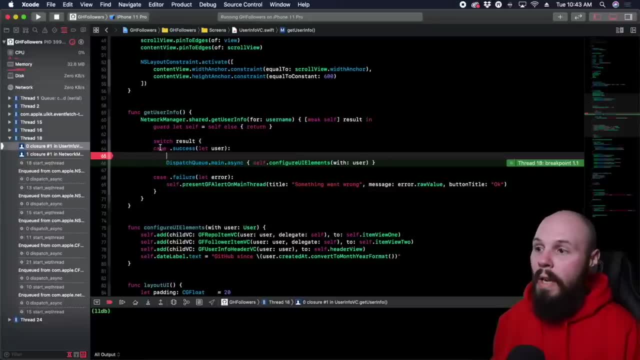 right here. So 65 it broke. So that means the code went into the success block of the switch statement. and then right here is where I stopped it. So now I can see: Hey, I have a user. So here in my debug console, let me scroll up here. 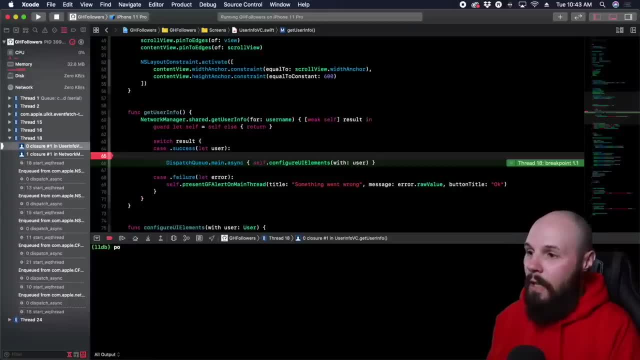 I can do a PO for printout and I can do user because I have the user right here. It depends on what scope you're in, but if I print that out now, I can see all the information about my user right here, right? 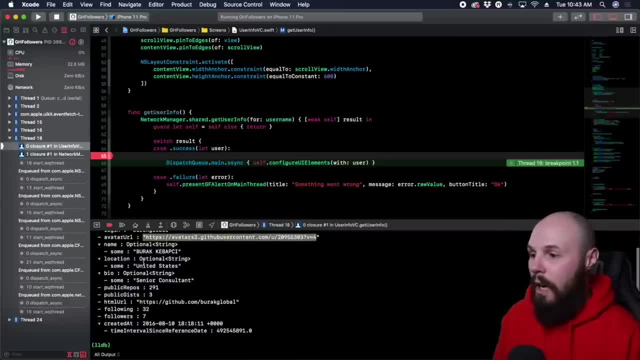 So there's the login. there's the avatar URL that we're pulling in. Uh, there's the location: United States. right, There's his bio: senior consultant. how many repos? right? All the information about that user struck that you may have seen in previous videos. 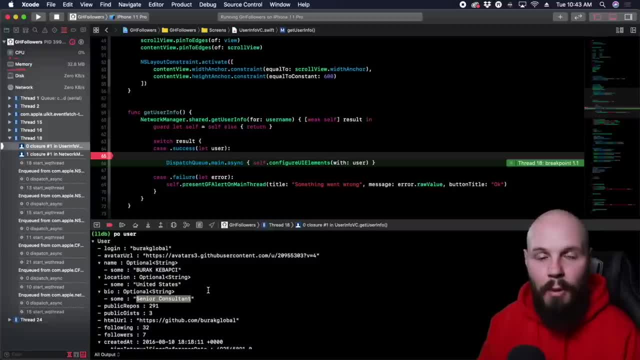 is right here live. So break points are a way to stop your program so you can like debug and see what's going on. Oftentimes, how you would debug is what would happen is that would execute and like: maybe the user information didn't fill correctly or, you know, something was wrong. 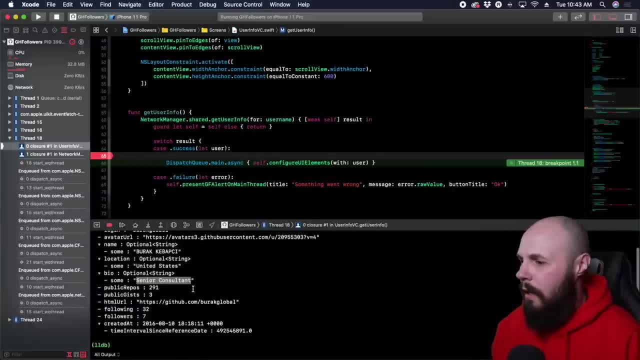 I would break, point it here and be like: okay, what user am I getting back? Okay, How am I getting back? Uh, and I would. I would be able to dive in and try to figure out what was going wrong with my program. 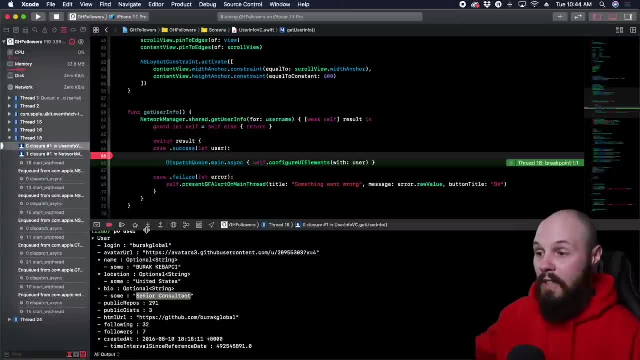 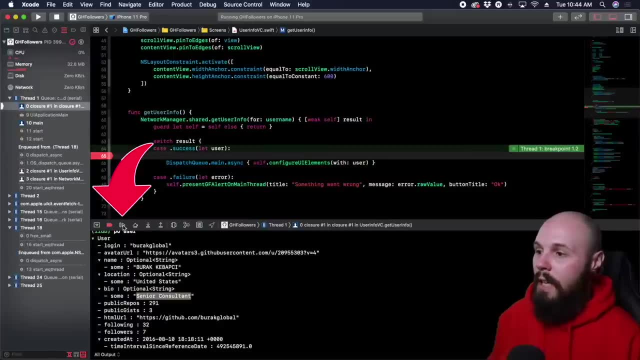 So that's the basic concept of a break point to help you debug. And now, like I said, I've I've paused my program in order to like rerun it, because I looked at this: Okay, Everything's cool. Now you hit this play button right here and that will run your app again. 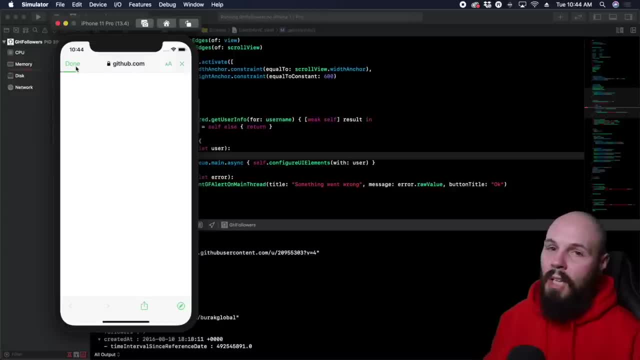 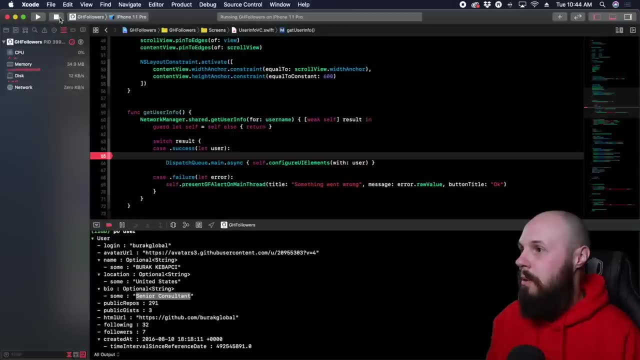 So now we're back to running in the apps, running like normal, but while you're stopped, uh, the app is not running, It's kind of like paused. So there you go. That is the basic break point. So stop, Stop the simulator. 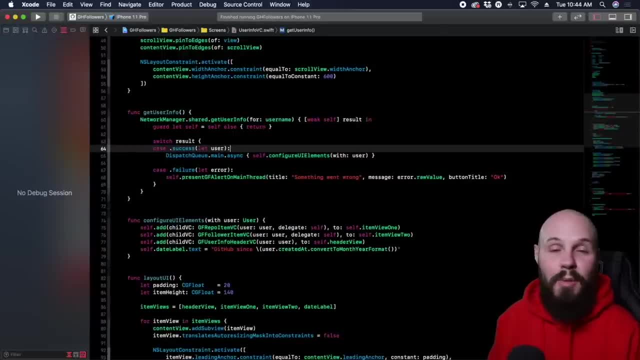 Get rid of the break point. Always make sure to delete your break points too, because, uh, sometimes you'll forget to leave them in, and then you'll be testing your app and it'll just stop and it'll scare you. You'll think something's broken, but you'll be like: oh I just I forgot to delete my. 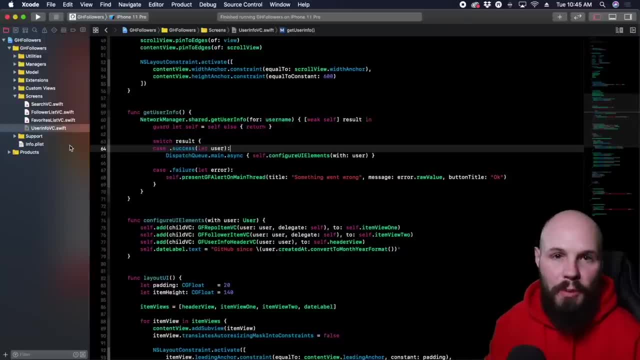 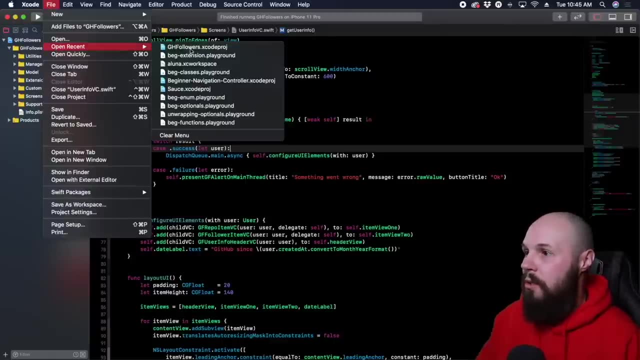 break point Now, this GitHub followers app that I've been showing you. we did this 100% programmatically in the course, So we don't have storyboards in this project. Uh, let me switch to a different project to show you storyboards here. 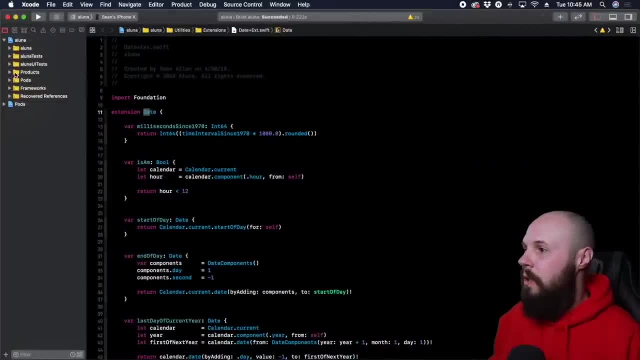 So open, recent open up a Luna and here we are in a Luna. So if I open that up, uh, you can see it go to storyboards. You can see I'm going to pull multiple storyboards, As you can see here. if you've worked with Xcode before, maybe you're used to working. 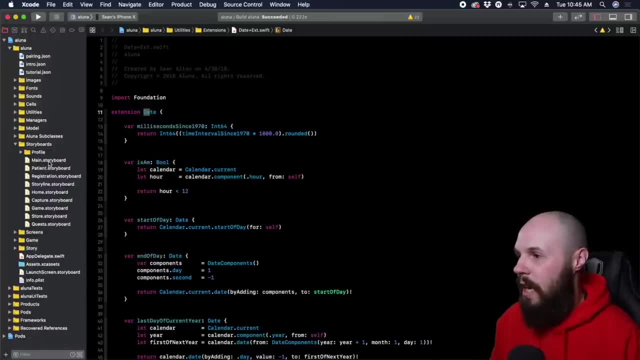 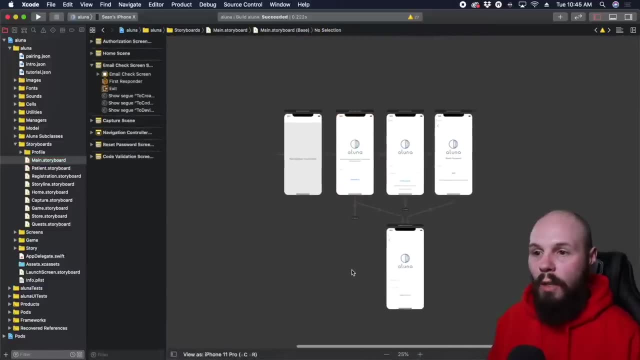 with one storyboard. We're going to talk about why you might not want to do that, So let me open up a storyboard here. Wow, That's big minimize Uh, so you can see. here is our uh, like our login screen, uh, for a Luna, and you can see. 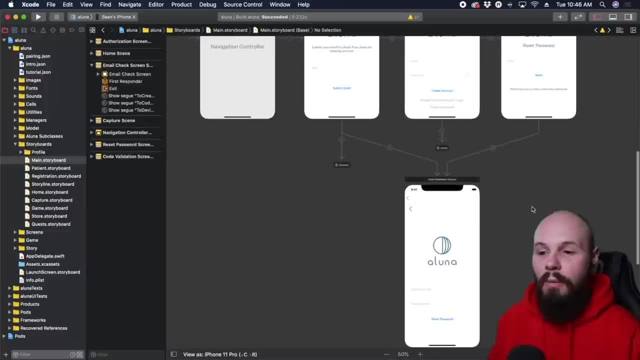 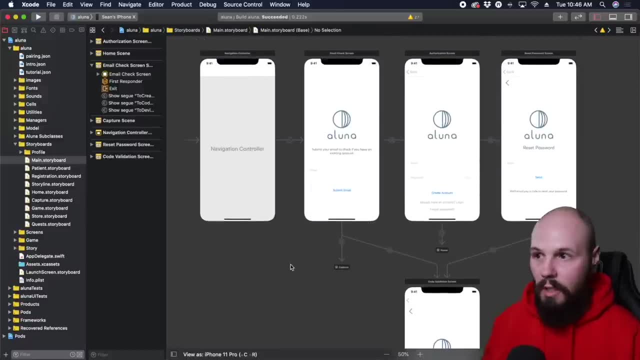 the pass here, right Cause we have a, like a reset password screen. We have an email verification screen, for reasons that have to do with the product, Um, so anyway, you can see. this is an example of a storyboard where you can see, you can. 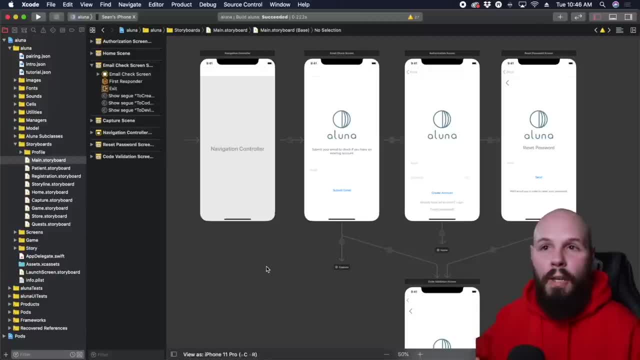 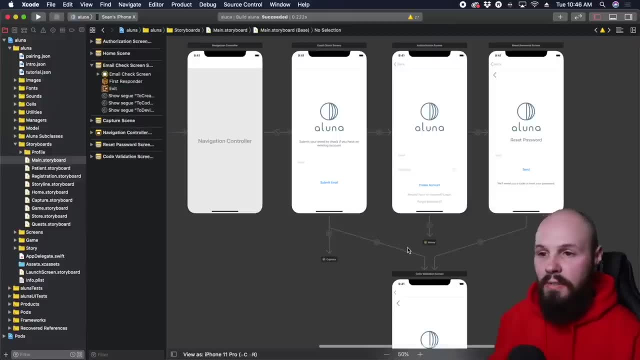 lay out your view control, Uh, which, to put it simply, they don't have to be full screens, but most of the time they're full screens. So in storyboard you can layer your view controller. You see, you can kind of make segues. 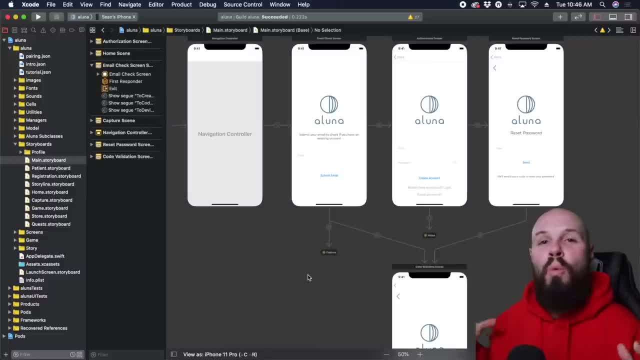 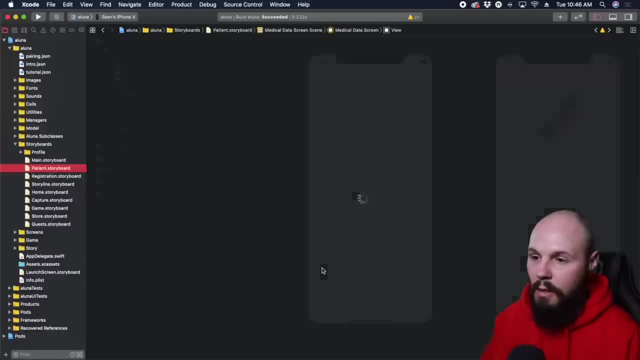 That's what these little lines are called to attach each view controller. It's a very visual way to lay out your app, And I have my the different sections of this app broken out. You can see. here's the patient storyboard. This is probably going to be huge too. 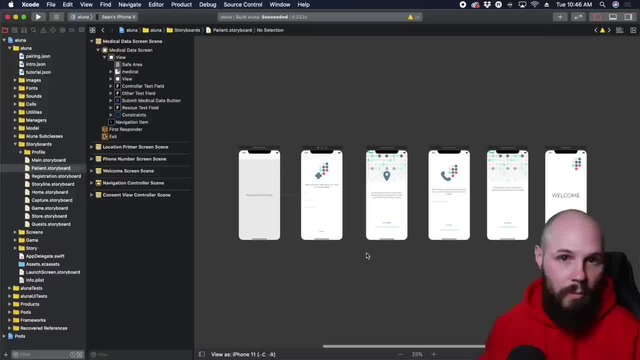 Yep, So this is our onboarding right, Where the patient is giving us like their medical information. by the way, this app has to do with like asthma for children. So there's like: what kind of? What kind of inhaler do you use and all that stuff. 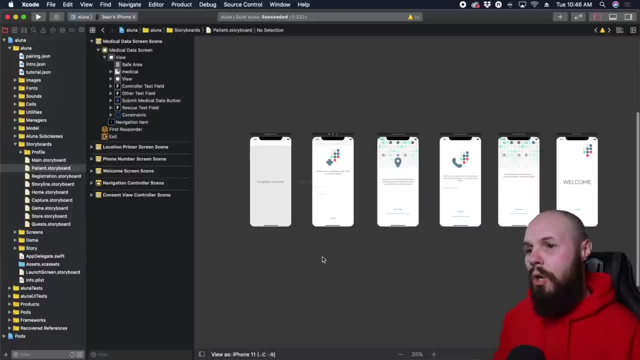 Um, but this is like our onboarding section, So, as you can see, a lot of beginners like storyboard cause they can visually see their app. However, there is a bit of a debate that I have a whole video on: uh, programmatic versus. 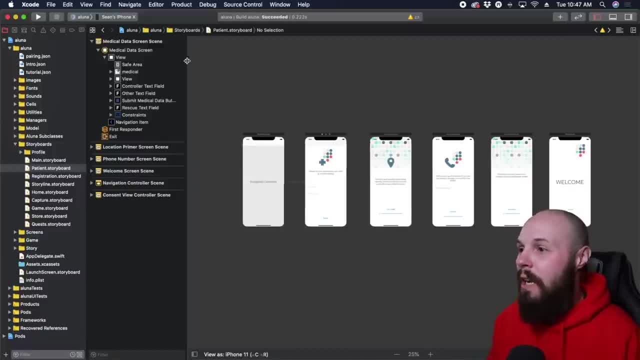 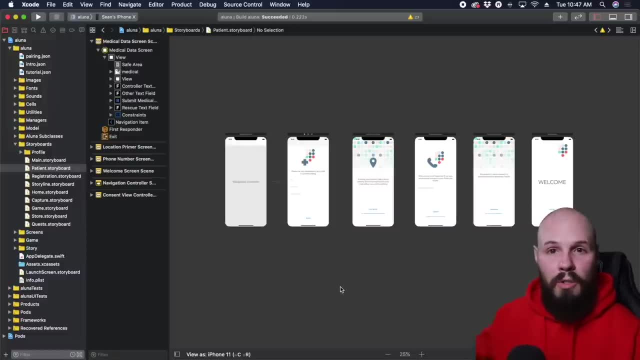 storyboard. but I'm showing you uh the storyboard here, and I'm just showing you what it is, because in the next video, where I talk about all the components of UI kit, we're actually going to be using storyboard, So you're going to get uh more exposure to that in that video. 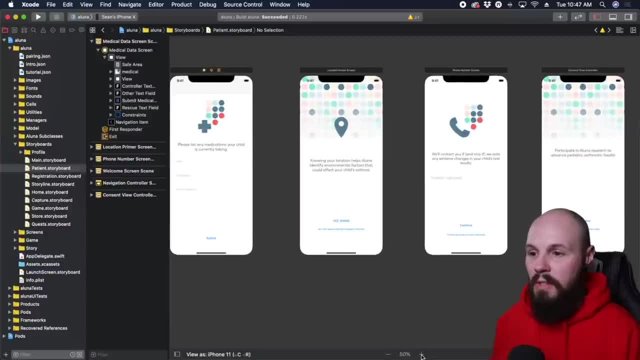 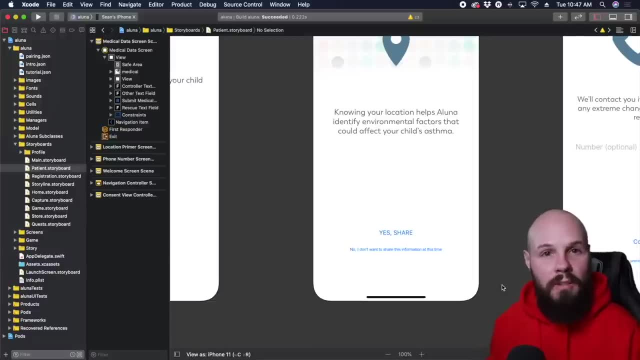 And real quick, I'm going to zoom in here right on these, like these buttons that you see, um not sharing your location. Now you see they're just blue buttons. Well, remember how we had that custom GF button. that was a subclass of UI button back in the 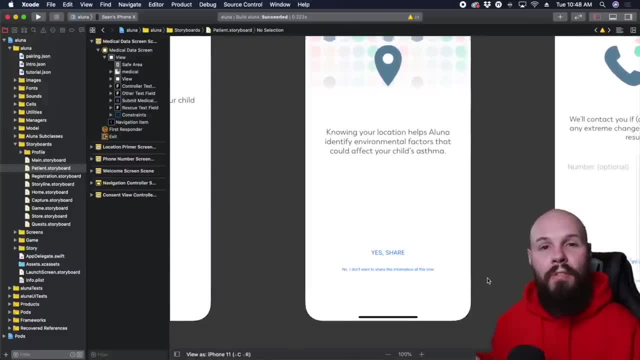 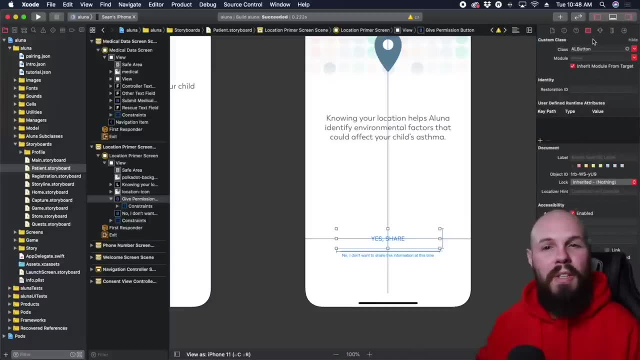 classes video. What I'm trying to say is storyboards don't always have to look exactly like they do in the app, For example. this you'll see when I click on this. I'm going to open up the right panel. more on this in a later video. where you can see this is a class of AL button, right. 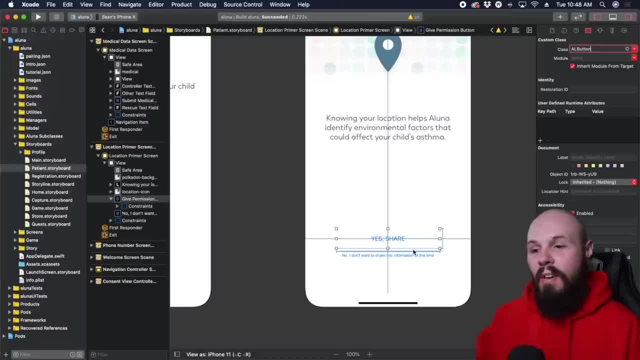 So that is a custom button that we have, that will you know. round the corners, give it a background color, Change the font, but on the storyboard all you see is this blue button. So don't worry if you didn't follow that. 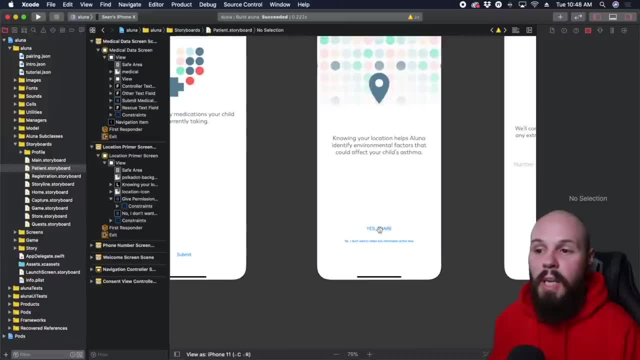 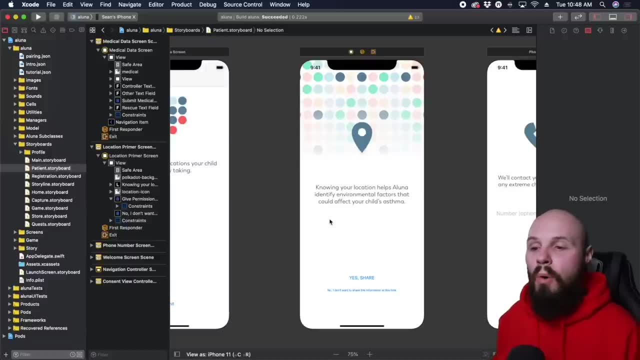 The main point I wanted to show you was that you know, just because you see a blue button here on the storyboard doesn't necessarily mean that's what's actually going to show up in code. So again, the main point is: what's on the storyboard may not be an exact representation. 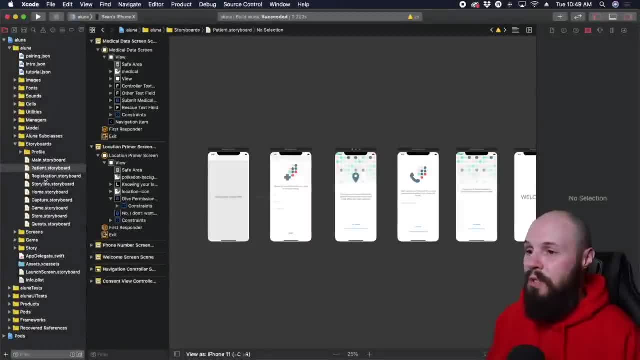 of what's on your phone. Now, like I said, this project is an example where we use, you know, multiple different storyboards. My rule of thumb- as you can see, we're kind of breaking it here sometimes- is that: um. 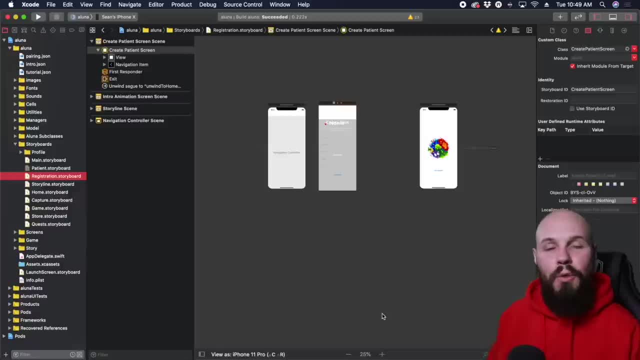 your storyboard. You can have three to four or five view controllers on it at one time, And the reason being that just separates things out and makes it easier to work on, especially if you're on a team. um, you can have this nightmare that you see here, that, if it's 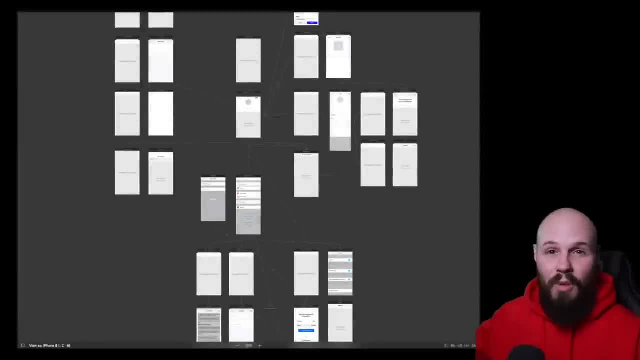 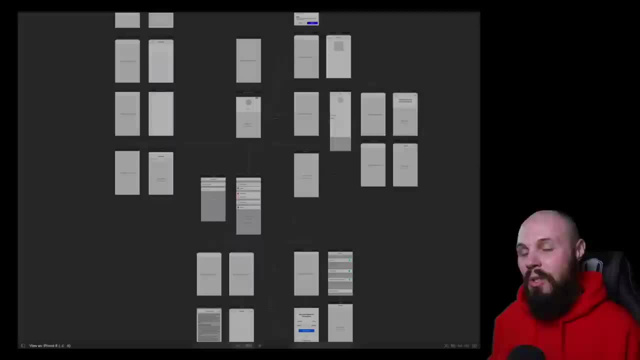 just one storyboard like look at this in your whole app is on one main dot storyboard. It becomes a nightmare to deal with, Uh and again, especially if you're working on teams. um. so anyway, one big takeaway: use multiple storyboards and keep them small. 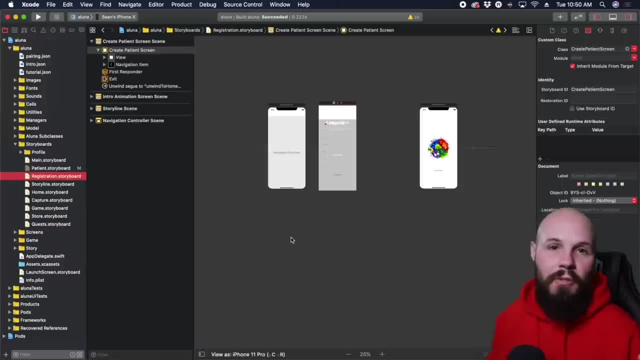 If you choose to use storyboards- And again, we're going to dive more into storyboards in future videos when we build our apps, So we will definitely get more practice using them. again, just an overview video. The last part I want to point out about Xcode is this project: uh settings part. 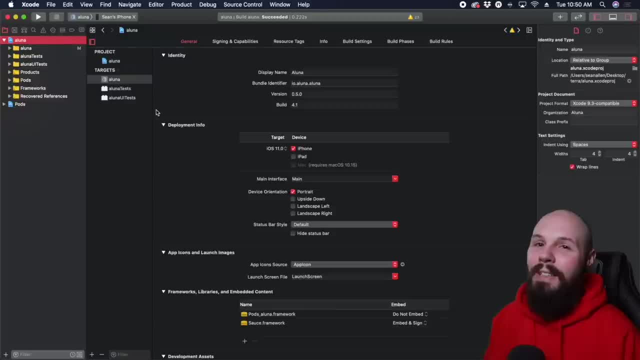 So, uh, this, don't worry too much. you know this is going to be confusing. This still confuses a lot of like even advanced developers, but this is where you have your. uh. well, this section is pretty straightforward, but you can see other sections will be tricky. 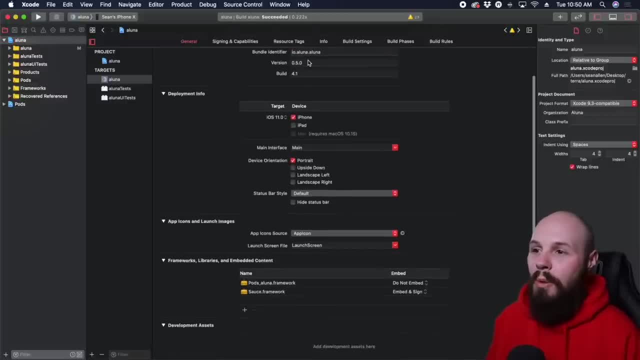 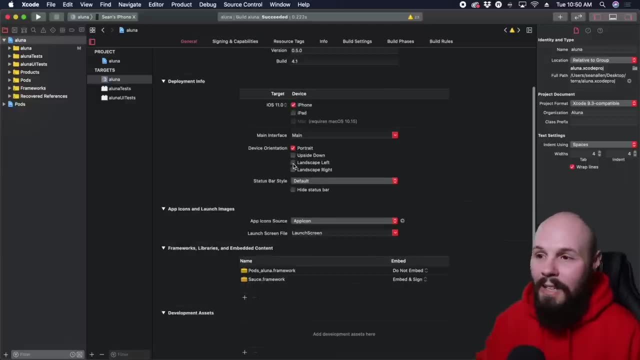 This is where you have like your display name on the app, What version number You know if you want to have it for the iPhone, the iPad or the Mac. uh, portrait mode, you can escape disable landscape, left or right. 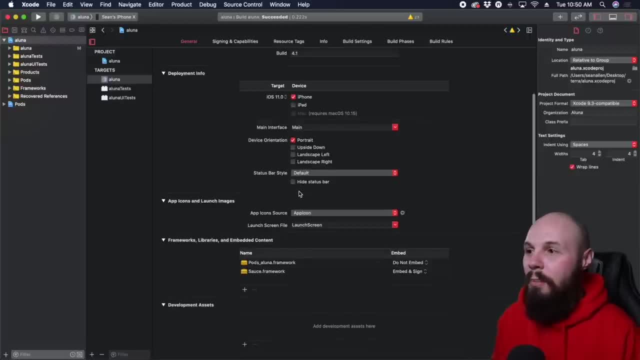 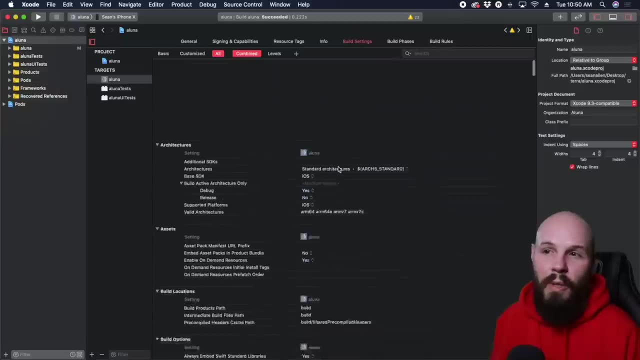 Right. If you only want your app vertical, you can disable that. So this is like the basic settings, but, as you can see, you get signings and capabilities, build settings right. This is just. this is where you get really into the weeds again. 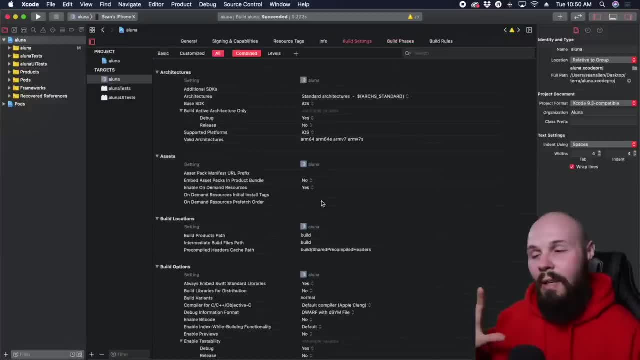 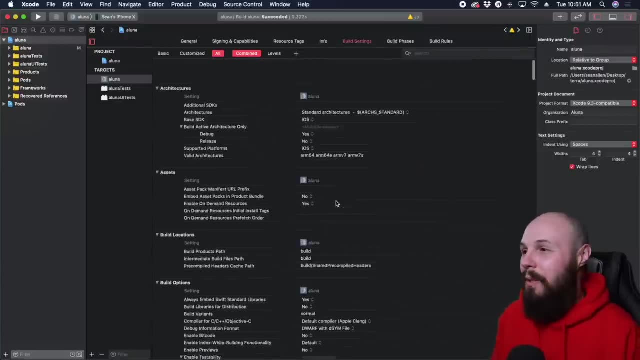 Don't worry about like understanding all these build settings and build rules. Um again, a lot of even experienced developers shutter when they get, when they have to deal with something on this screen right, It can be a real nightmare. but anyway, I wanted to point out that section to you. 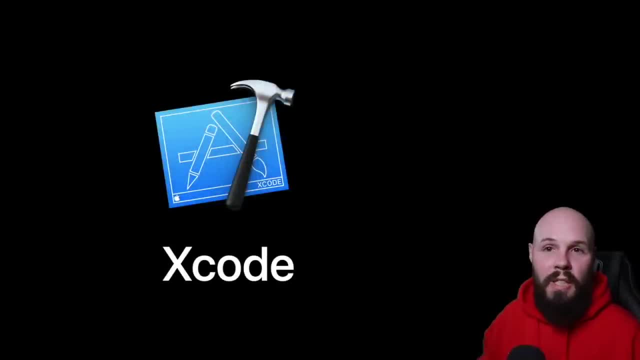 Um, but that wraps up the overview of Xcode. Again, we're going to be using this pretty much the rest of the course, uh, as we build our apps, So we're going to get a lot more experience with it. Just wanted to show you the main components onto the next video. 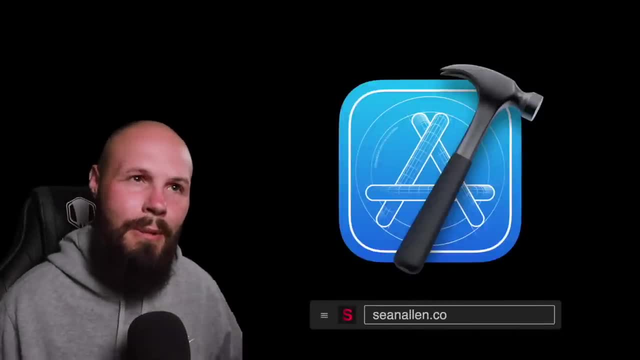 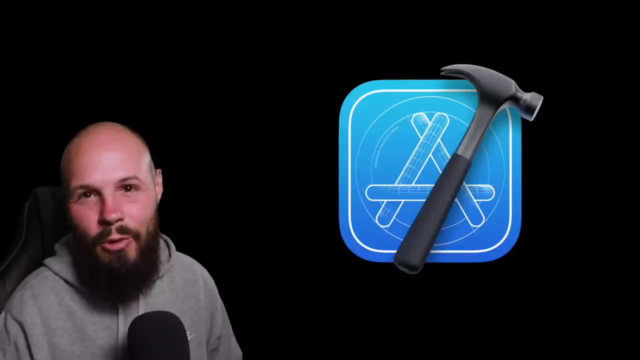 Today I'm going to show you some of the highlights of what's new in Xcode 12.. Now I say highlights because anytime we get a brand new Xcode there's a ton of little things that they add. for that There's a link to the uh release notes. 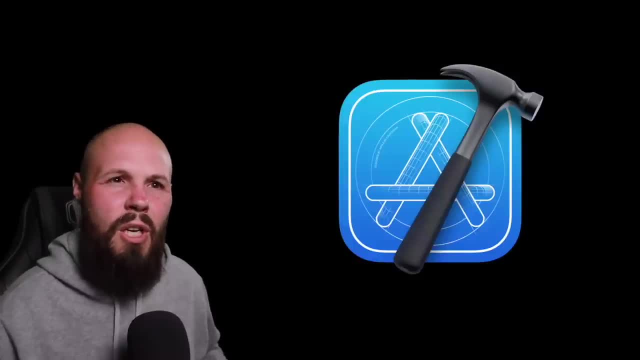 Go ahead and scroll through that. It's very long, have a ball. But for this video we're going to focus on what I feel are some of the more common things that people are going to deal with on a day-to-day basis. 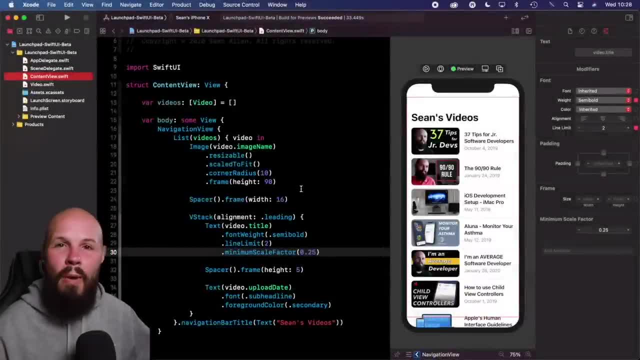 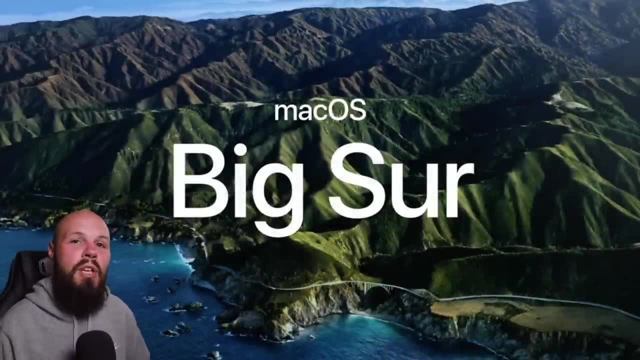 First, let's talk about this new look and feel of the design. Now, right away. I am on Mac OS Big Sur. I am risking it a little bit on the first beta. uh, on a question I got a lot on Twitter is: do I need to have Mac OS Big Sur in order to download the Xcode 12 beta? 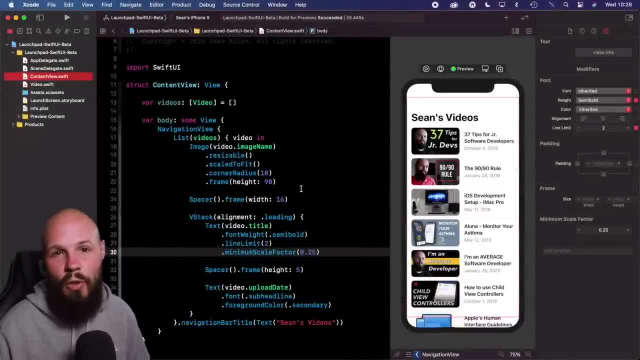 The answer is no. You can still be on Mac OS Catalina and download the Xcode 12 beta. Uh, you won't get this redesign, but you'll still be able to get all the features. So if you look here, the you know the play button, the stop button icons got redesigned. 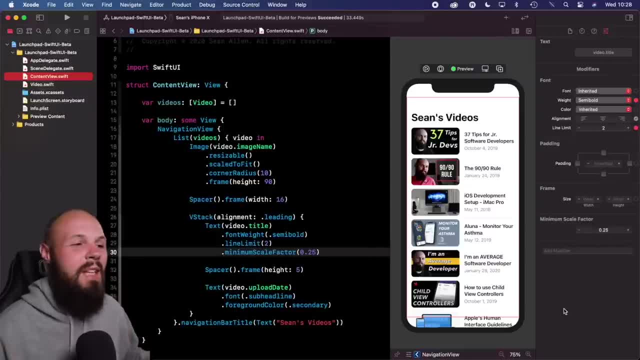 over here on the right We have the inspectors. you know they're more spaced out. They got redesigned Um the sidebar here. one thing that helps especially for me and maybe people that you know- poor vision, I guess- is when I'm doing these videos I got to like blow my screen. 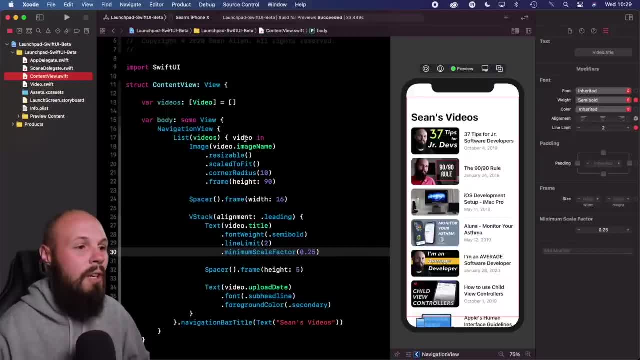 up so you can see it. you know, on your phone or on your computer or whatever. Now when you're doing your font, your code, you can do command plus and command minus. That's been around for a while So that's easy to adjust. 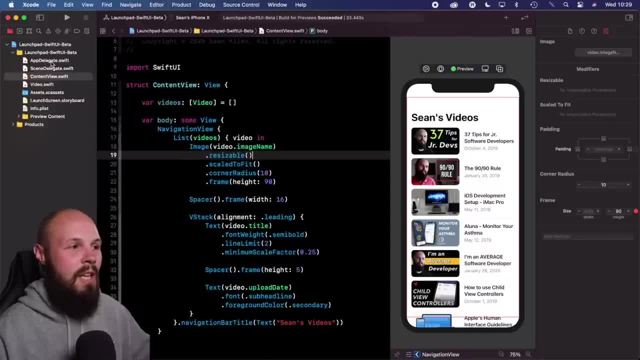 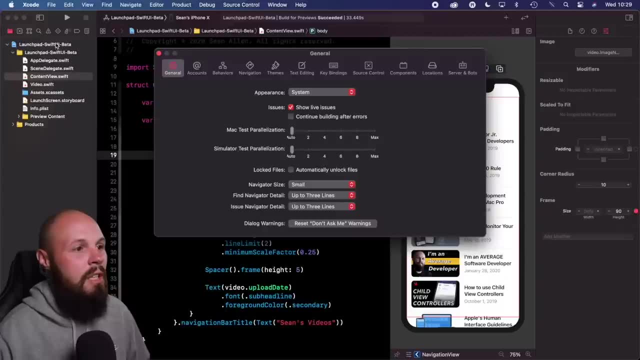 However, the navigator here on the left. you can never adjust that size, Even though I have like my largest font based on my display settings. Now you can change that. So if you go to Xcode preferences here in general you can see navigator size right. 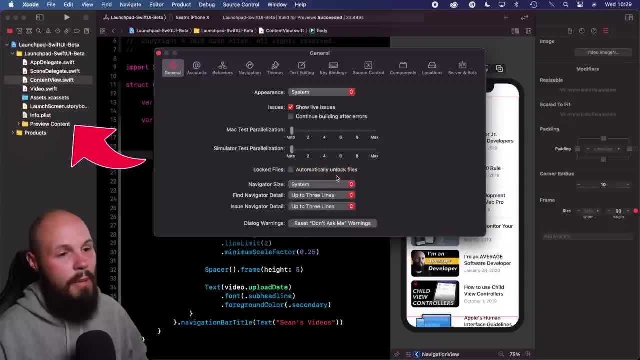 now I have it set to small. Uh, you can set it to whatever the system is. So you can see that made it a little bigger. Now I can also set it to large and if you watch it, it's going to get a little bigger. 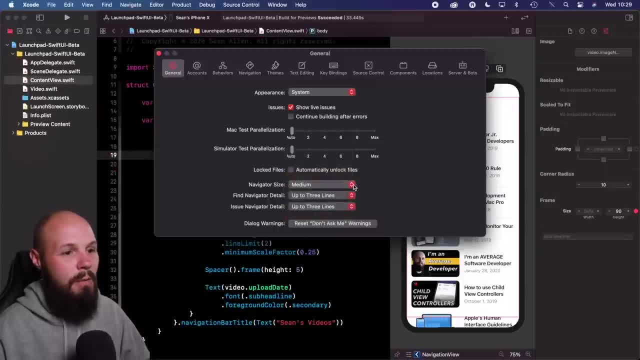 So see, it's not like a crazy drastic change between small, medium and large. Like, to be honest with you, I kind of wish it was more drastic, Like going from small to large doesn't. I mean it feels different, but it's not a crazy. 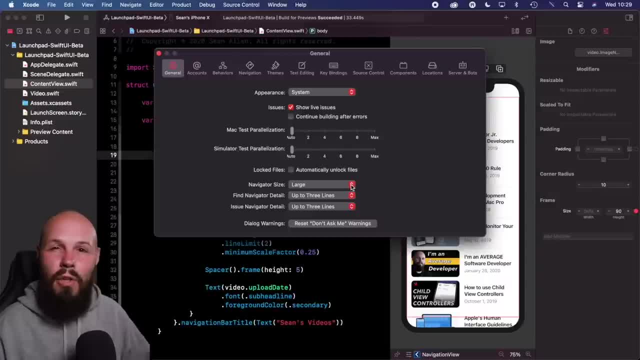 drastic change, But, uh, anyway, that's a. that's nice. If you ever felt your navigator was way too small, you can now adjust the size of that. I'm going to leave it on large for you, uh, for you watching at home. 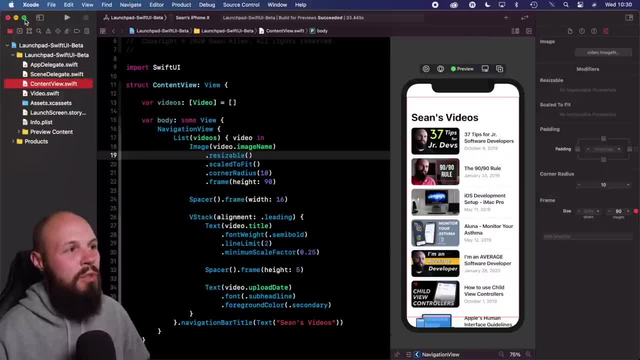 And speaking of sizing issues, those of you that work on laptops- if you go full screen right, you have these inspectors on the right and the left And if you're in SwiftUI, you got the preview, Like I'm on my iMac 27 inch screen. 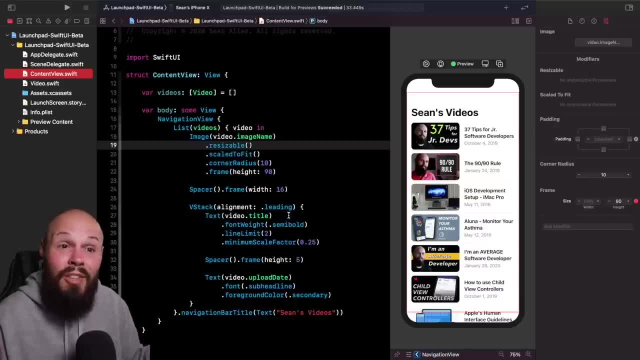 So things are spacious, but on your a 13 inch MacBook Pro, like things are tight, So oftentimes you know you're on your MacBook Pro. you're on your MacBook Pro, you're on your MacBook Pro. You may click these icons in the left to get rid of the navigator and get rid of the inspectors. 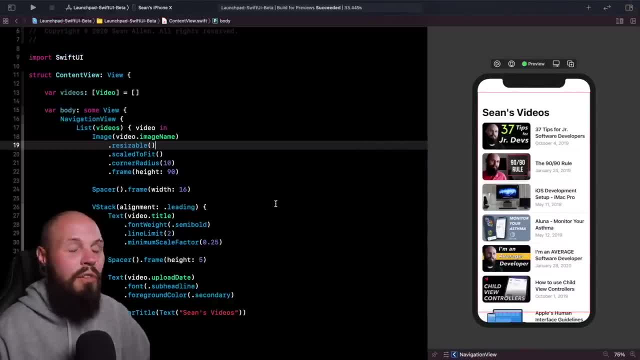 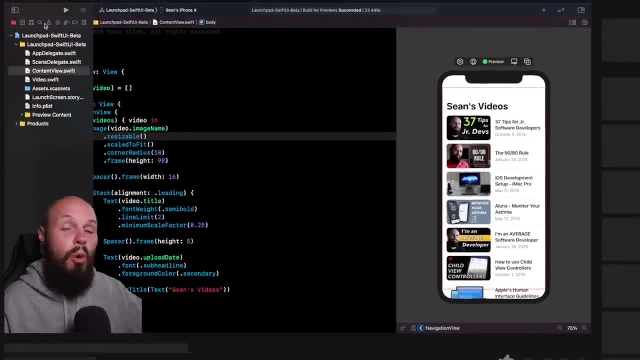 just to have more room to work. Well, the cool thing in Xcode 12 is now: if you have your inspector hidden, just slide your cursor to the left and it slides out. You know, you can navigate, you can search, you can do all this stuff here that you normally 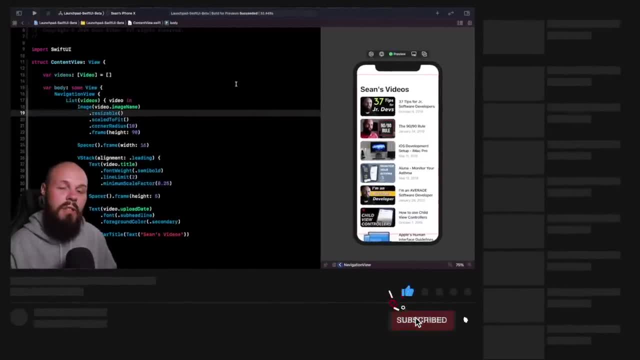 could if that uh navigator was always showing and then you go and it slides away. It doesn't work with the inspectors on the right. Uh, to be honest with you, I don't know if that's intended or if maybe that's coming. 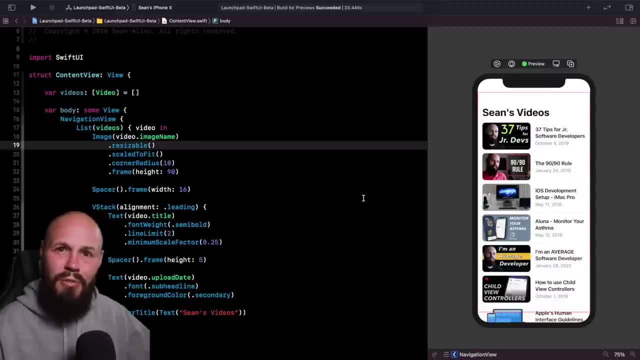 in a later beta version. uh, I recommend, if you're downloading like the official version of Xcode 12, not the beta, Give that a try Again. I don't know if that's intentional or not, but the inspectors don't slide out. 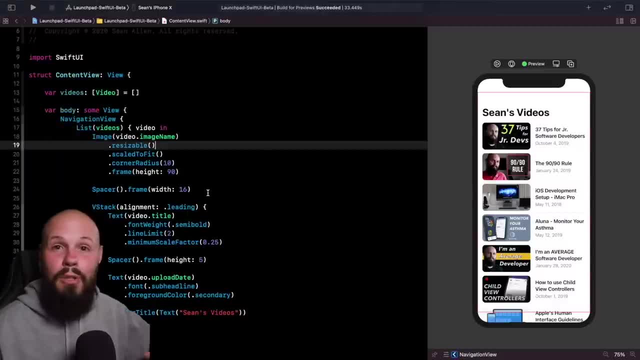 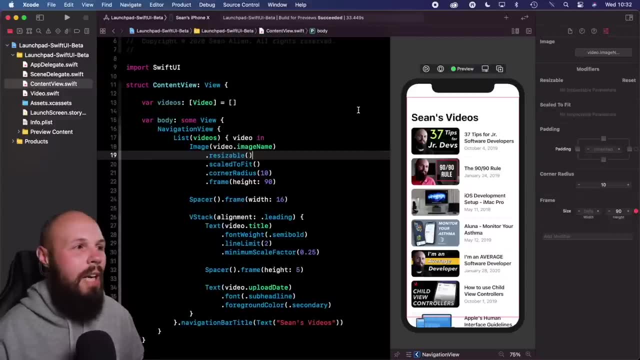 but the navigator does And, like I said, if you work on a laptop and you need that screen, real estate, uh, this is, this is a lifesaver. Now let's talk about app creation, because now you can create multi-platform apps. 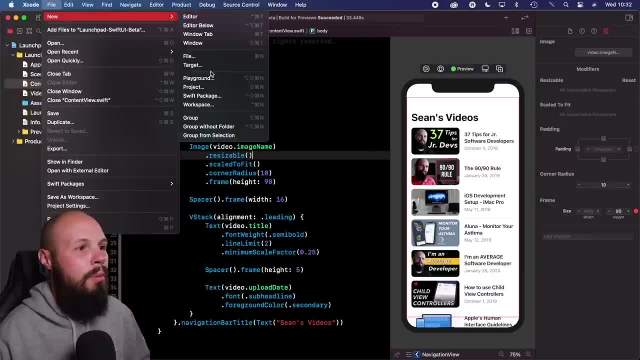 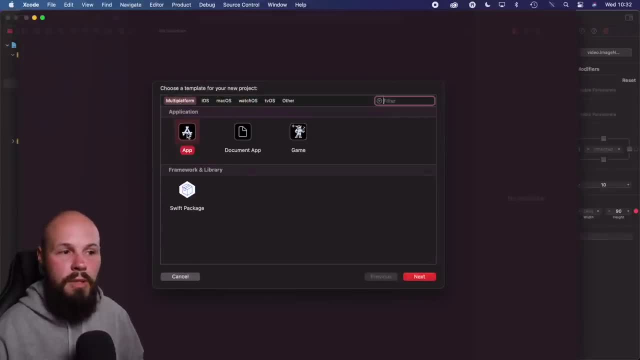 So we'll create a little test app here. So file a new project and here you see you have up at the top, multi-platform iOS, MacOS, et cetera. Let's do multi-platform and just make it an app and call this a test for. 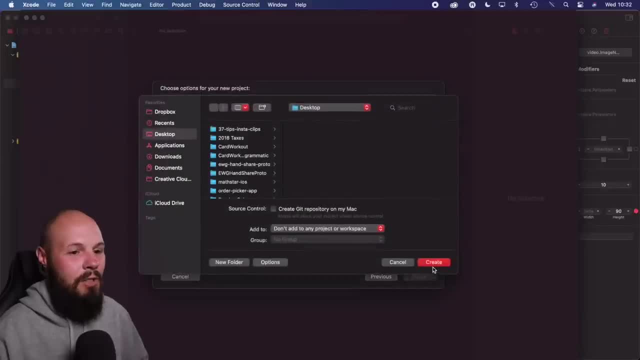 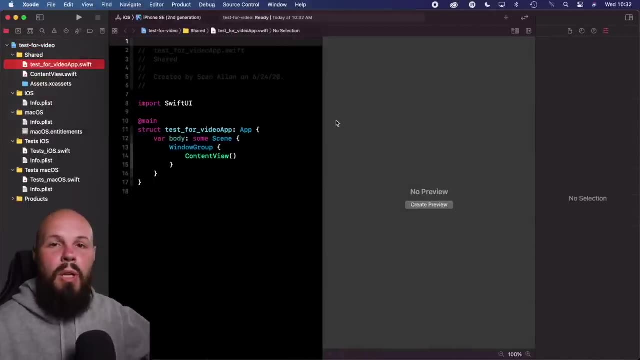 Video Cool. Hit next. Uh sure, Save it to desktop and make these windows bigger here, while this is, uh, updating all this stuff. This is just a sample. uh, you know a blank Swift UI, So what you'll notice here is app delegate- scene delegate. 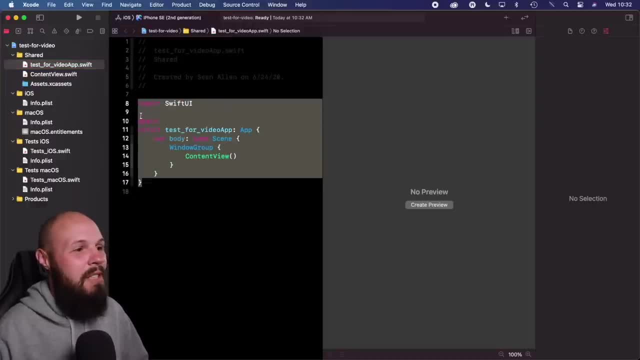 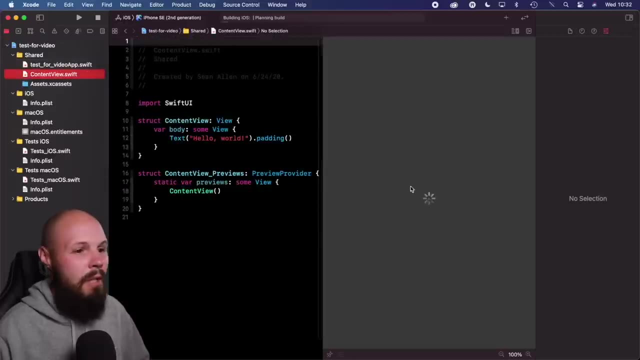 That's not a thing anymore. This is basically replacing your app delegate and scene delegate with this uh at main uh here. So basically this is now your uh app life cycle, So that's pretty cool. Uh, let's get this. 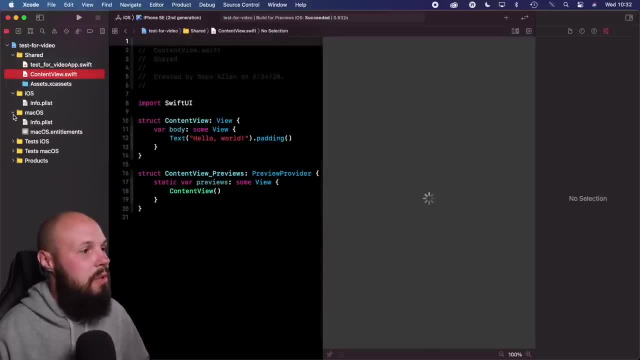 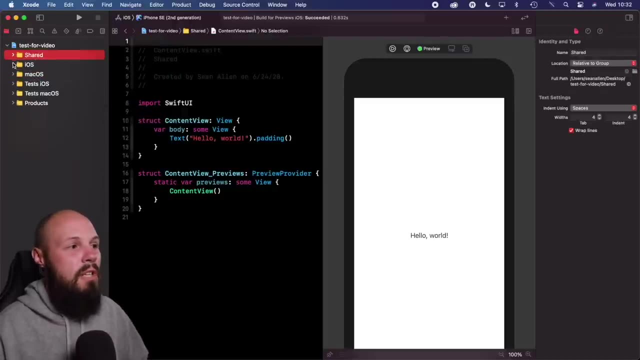 This is just the basic content view, but what you'll notice here- let me start minimizing some of these folders, So you can see- is I have an iOS folder, a MacOS folder in a shared folder. So the purpose of this is the shared folder. 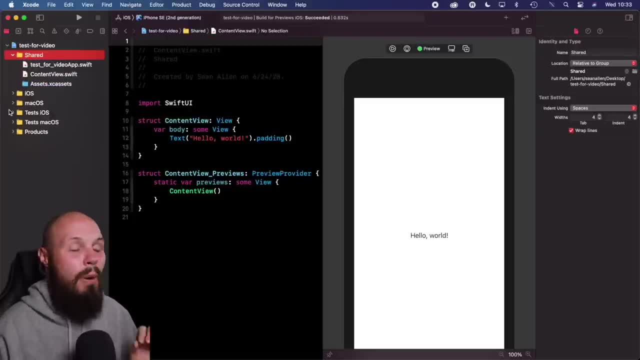 That is all your common core UI for your app. However, if you have something that is, you know, obviously an iPhone screen and a Mac screen are very different, So your UI may need to change so you can have specific files, screens, whatever views uh. 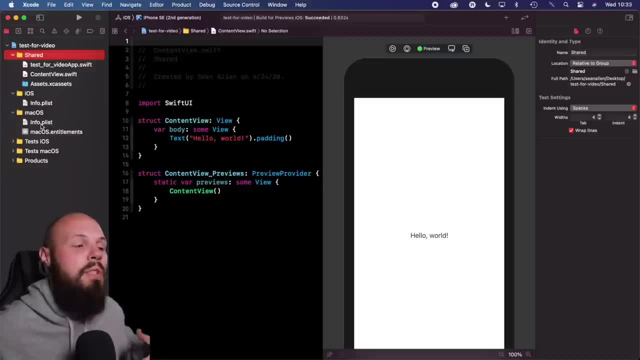 for iOS and MacOS in these folders. Okay, So that'll help you build these multi-platform uh apps. And the last thing I want to mention about app creation or, I guess, app updating: uh, as you know, Apple Silicon is coming out. 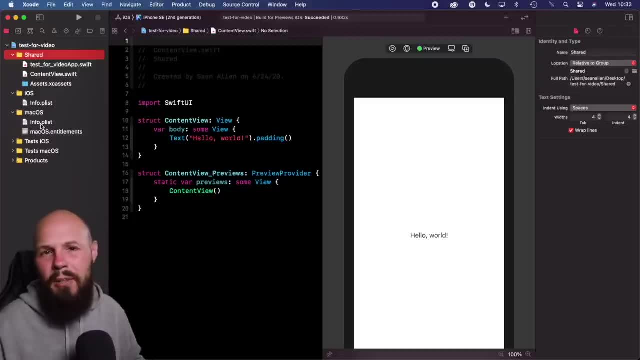 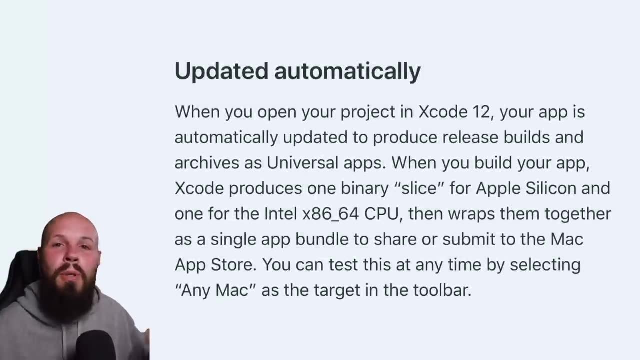 If you didn't see a WWDC. however, that is going to be a transitionary period, So your apps on the Mac are going to have to support Intel Macs and Apple Silicon apps. So the great thing about Xcode: as long as you build your project in Xcode 12, it's automatically. 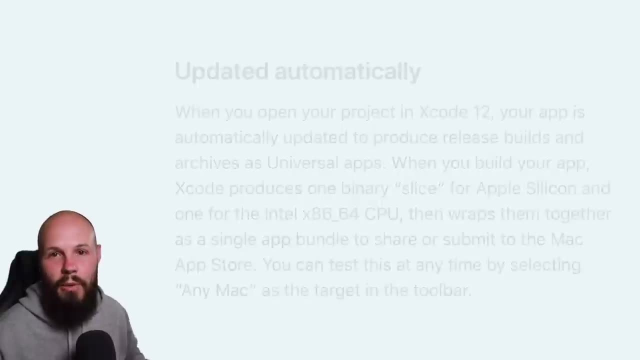 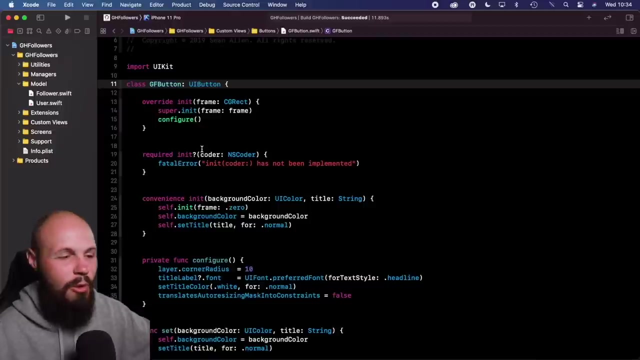 going to build both binaries for for both platforms. So you're going to be good to go there and let's switch apps to get up followers here. And I'm doing this because I want to show off document tags. Uh, because I need folders and all that stuff with a lot more files in that previous app. 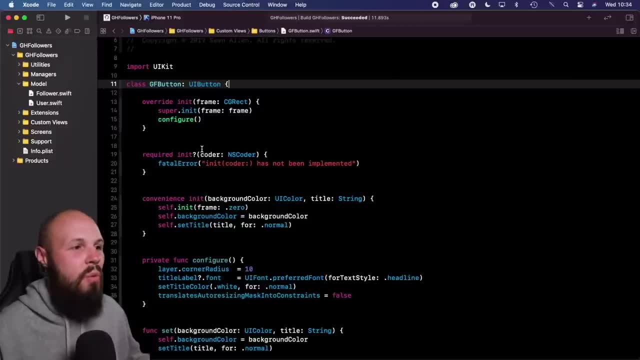 pad. So, uh, now we're in the kind of like the workflow section of the video where I'm going to show you some new cool things you can do with your workflow. So the first thing is document tabs, which is a nice way to organize what you're working. 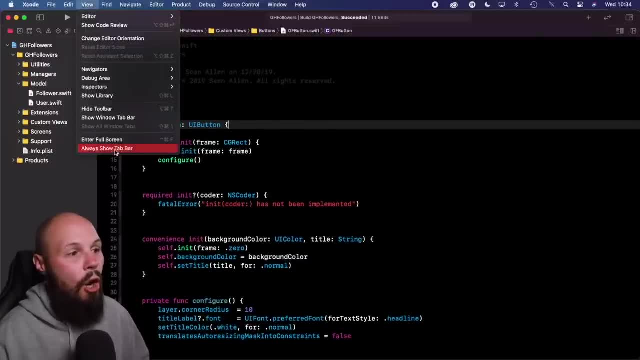 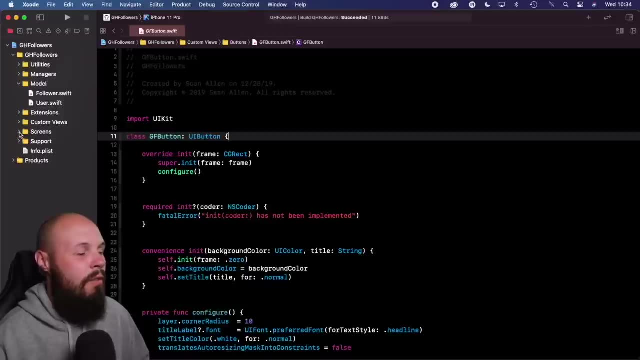 on. So in order to show the tab you do view uh, always show tab bar And then what you see at the top here, GF button. I get this tab here now on uh, whatever file I want to click. 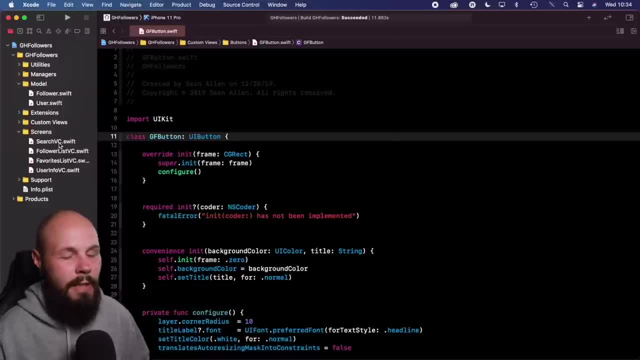 If I you can option click it or you can double click it. I'm probably going to end up double clicking it 99% of the time. So double click: search VC. There it is. Now you have this tab. double click follower list. 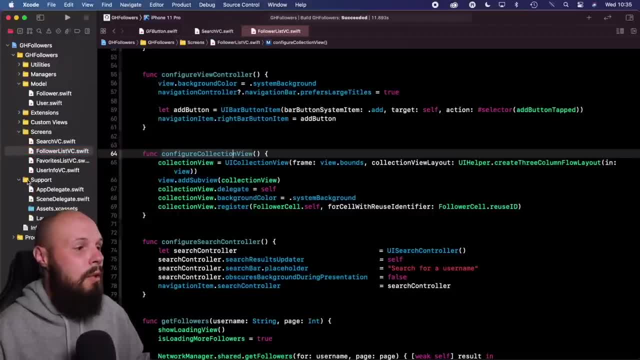 Now you have all these tabs, and it doesn't have to be swift files. Let's go to you know my XC assets? Cool, Let's go to my P list. There it is. So now you can just go through these tabs at the top, based on what you're working on. 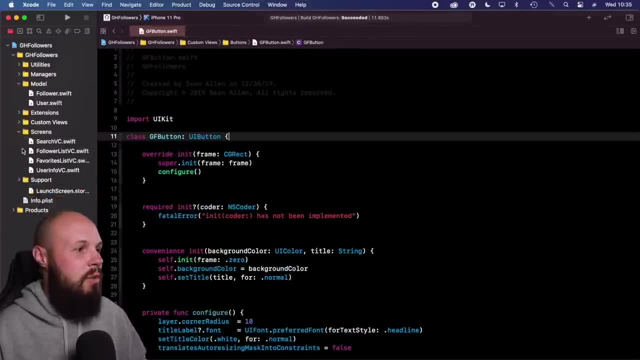 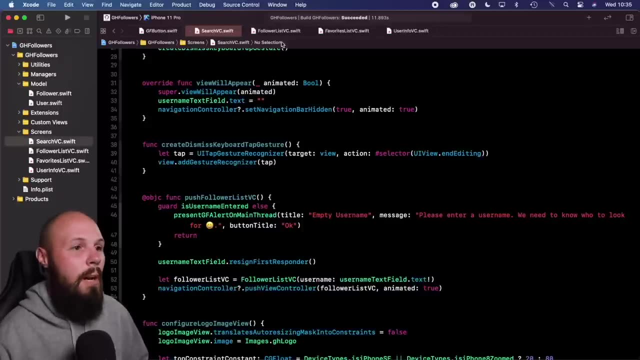 And if you want to like a whole section, like I'm closing these tabs now- like, say, I just wanted like all, all my screens in this app, I can drag the screens folder into the tab and it opens up all in new tabs. 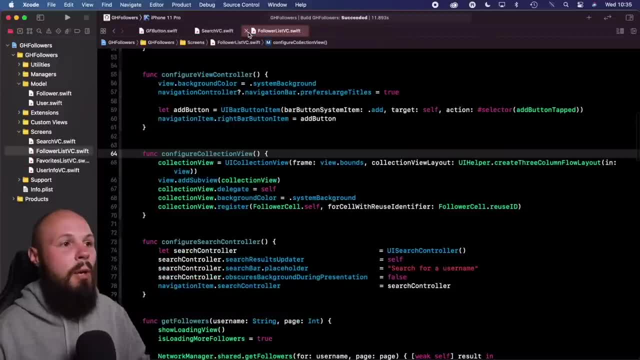 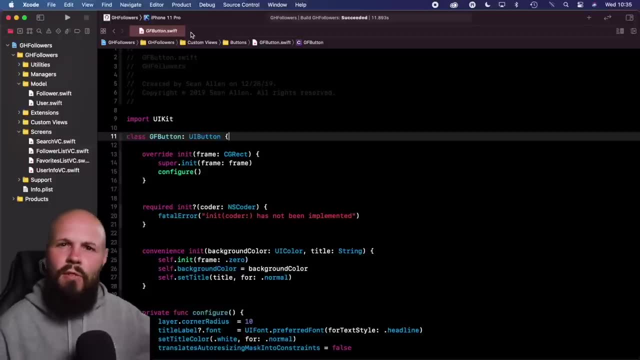 And I got all my screens In the tab as I'm working. So, like I said, it helps you organize what you're working on. And, speaking of that organization, you can have, like, multiple editors with different sets of tabs. So if I click this plus button on the right here, this pulls up another editor side by. 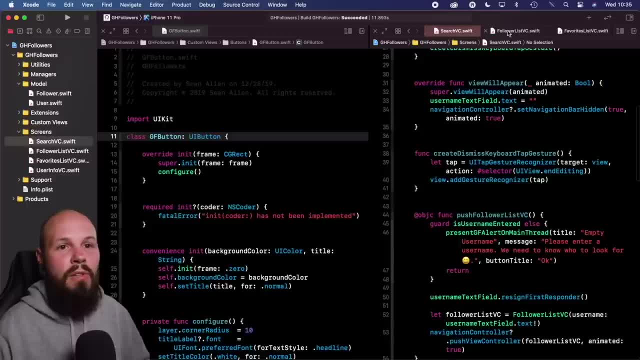 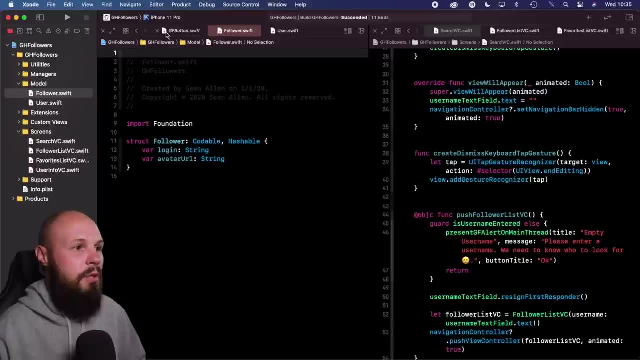 side. And let's say I want my screens on that editor. So there they are. I can get rid of the GF button one, So those are all my screens. And then let's say I want my model on this editor, right. 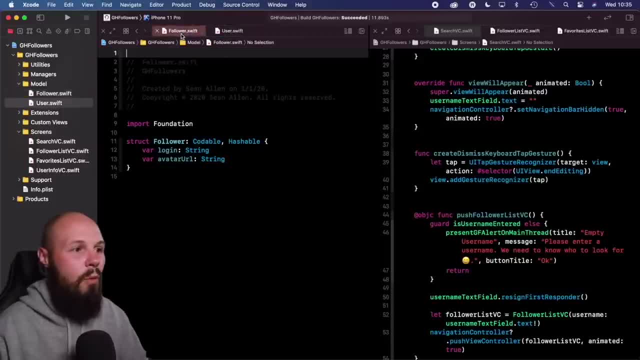 So I drag my model folder. So now I have in this editor I can go back and forth between my model objects, And then in this editor I can go back and forth between my model objects, And then in this editor I can just, you know, navigate through all my screens. 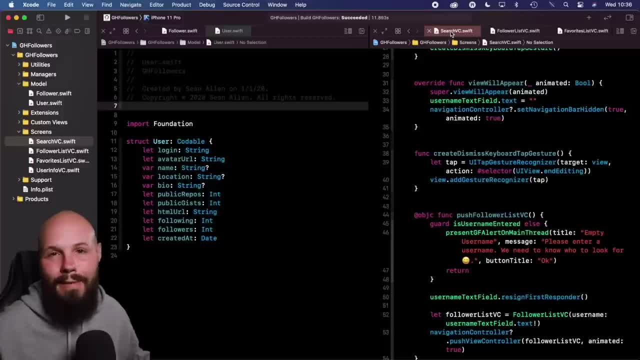 So, again, it's a nice way to organize. you know what you're currently working on at that moment, All right, So let's close out this editor, close out these, uh, these screens We don't need. we're gonna talk about code completion. 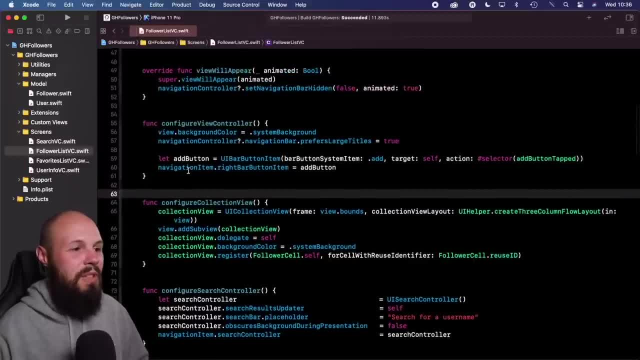 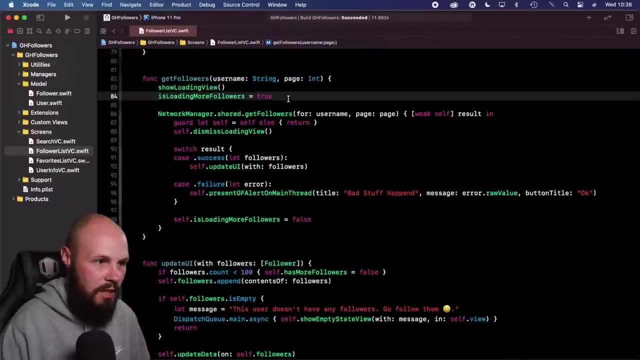 Now code completion is, um, I don't know, maybe maybe a little difficult to uh, to showcase, uh, here are the speed of it, but I'm also going to show you, like, the simplified results here. So let's do this. this network manager, make a network call here. 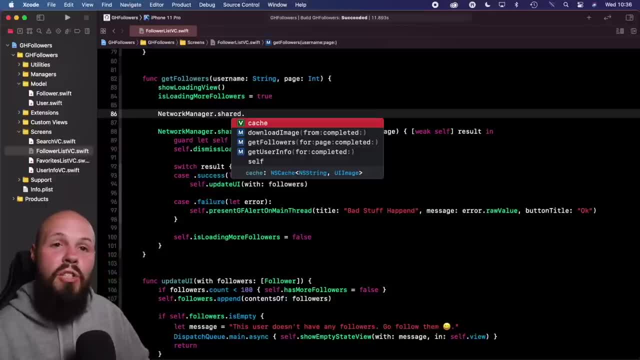 So network manager dot shared again. the speed may not be coming across, but what I can show you is: look at this, The simplified results. you know, sometimes you're getting that auto-complete and the auto-complete is like so long that it gets like truncated. well, here we just get very. 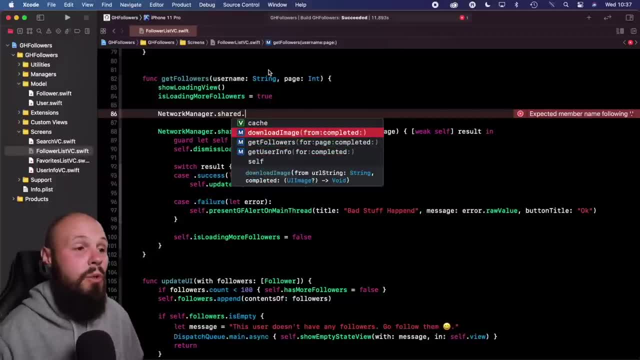 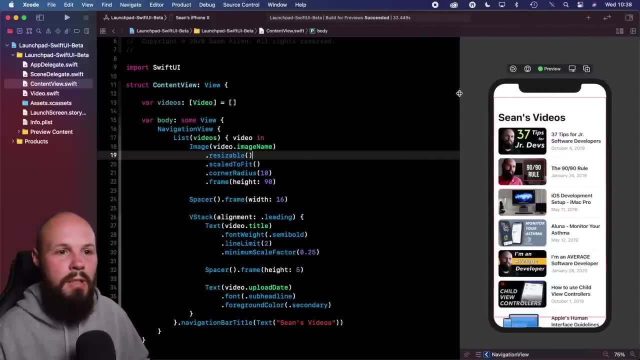 simplified results for our auto-complete. So that's also new in Xcode 12.. Now let's switch back to the SwiftUI app to show you some of this stuff they got going on in preview. I'm going to hide the inspector to really showcase it here. 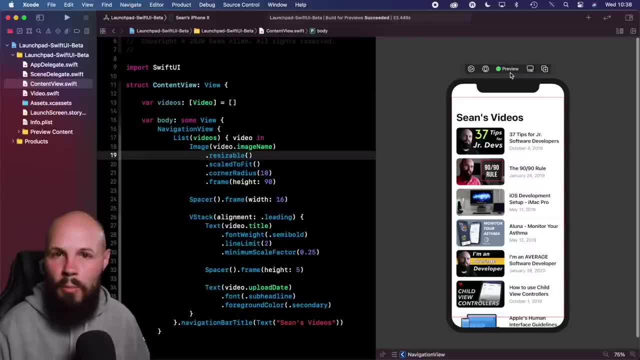 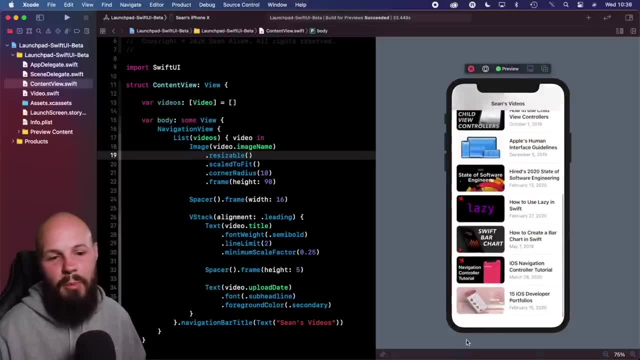 So you'll notice, above your preview you have this new preview toolbar, and this is pretty cool. It just puts things that you commonly use like just in a very convenient spot. right, You can run your preview right there. I mean, that was kind of below it, so that's not a huge change. 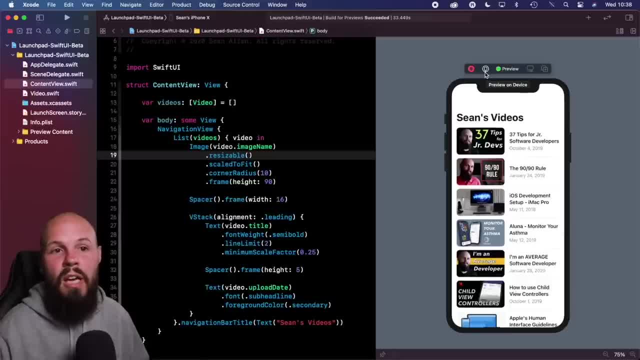 You can run it on device by clicking this button right here: see preview on device. This is the cool thing: You can quickly duplicate previews, Like before you would have to go down to your, your content. you know, preview type another. 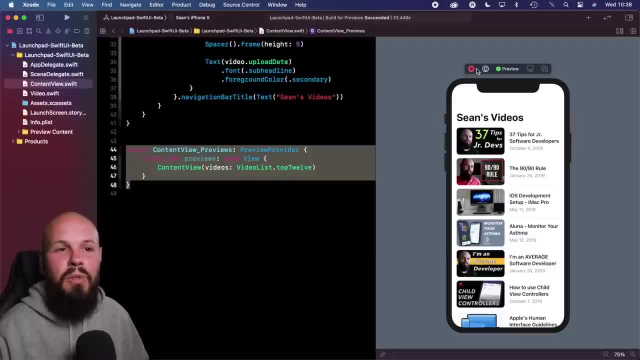 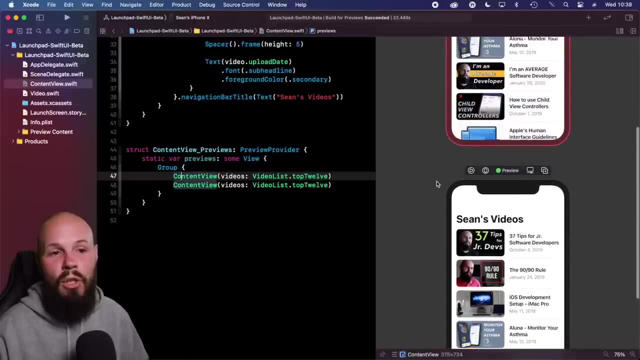 one out or add one, like a little little tedious. Now you can just we'll stop running this. Now you can just click on this duplicate, There you go. You see the code got added right there and you see I have another preview, and then right. 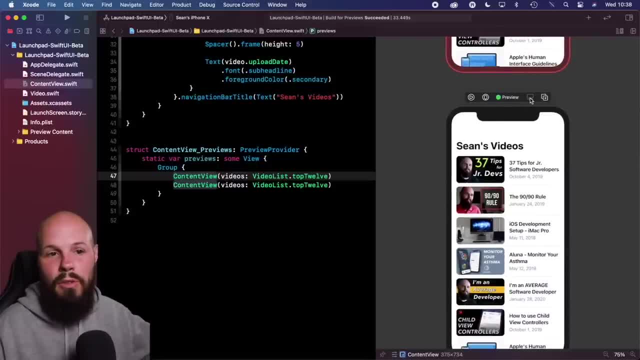 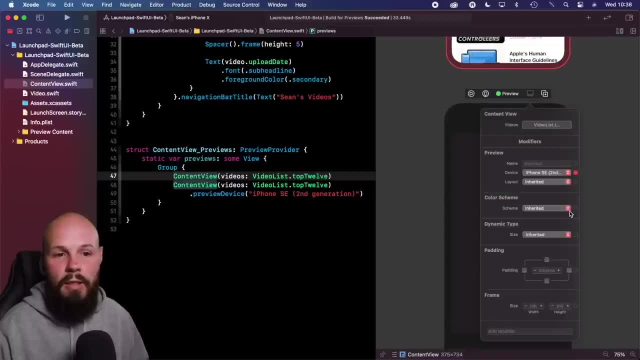 here you can adjust the environment of it and inspect preview- right, So I can go. look, a device can be. let's make this the iPhone SE second generation. Let's go with dark mode- right, So you can dynamic type. You know what? 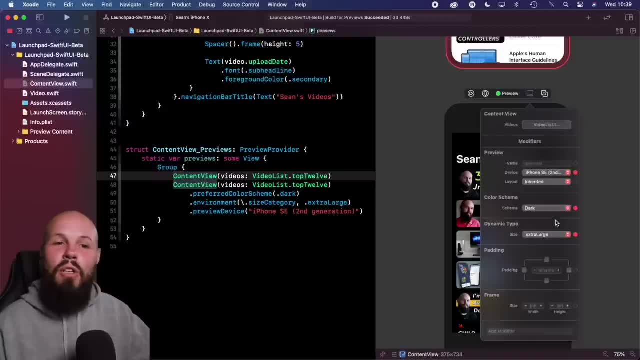 I don't even know if I did dynamic type on this app, but we're going to do extra large, right? So you can tweak. It's kind of like the environment overrides. You can tweak your preview right here from this toolbar right above it. 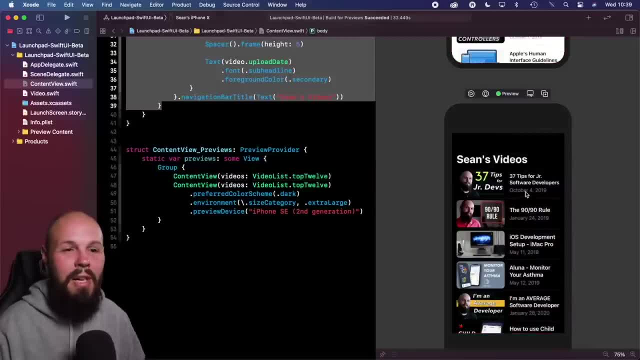 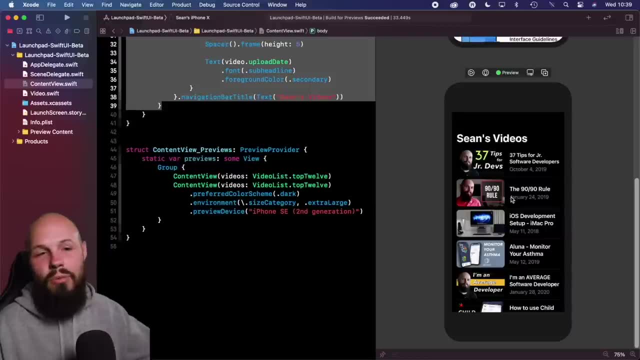 So it looks like I'm not really supporting dynamic type. This was a simple sample app, nothing crazy, but you can see in my previews I quickly duplicated it and I quickly adjusted the environment of it. Right, So real quick change the phone. dark, dynamic type, all that stuff. 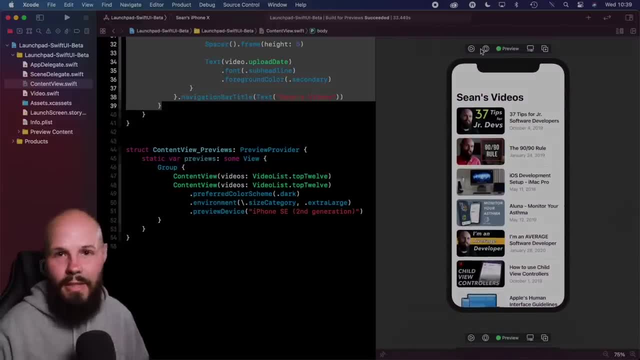 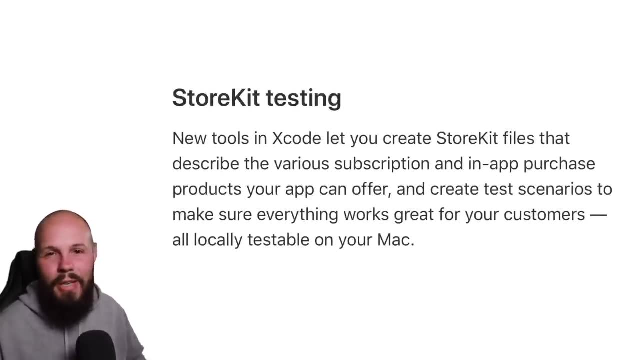 So, again, this preview toolbar that you see right here, very, very convenient. And, last but not least- I know a lot of developers rejoice for this- We have store kit testing. like store to testing used to be a major pain. Now you can test it without like deploying or staging your app right. 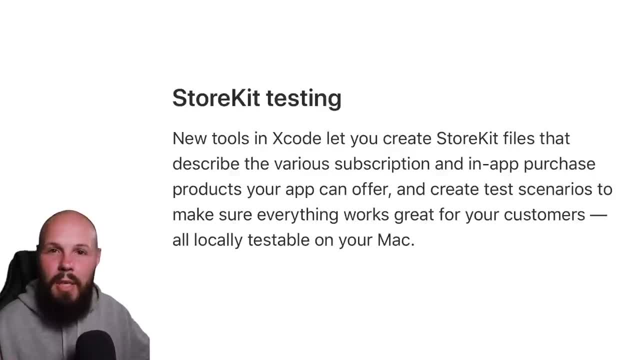 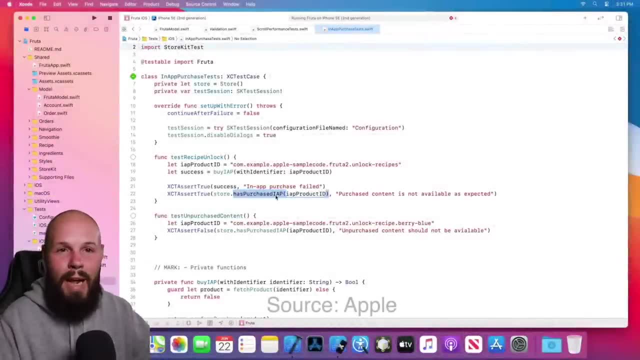 It's built right into the test, So I actually don't have an app set up with in-app purchases that I can like show you this. So I'm going to rely on the video from the state of the union address right here from Apple. 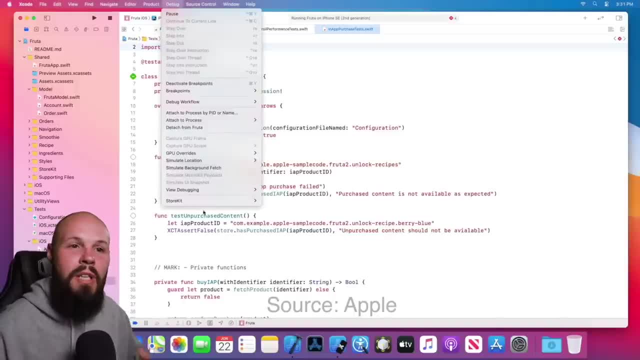 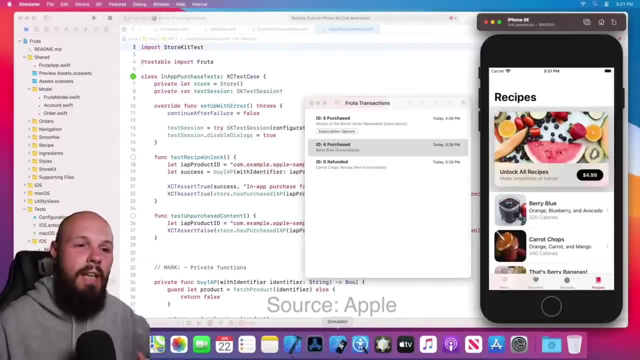 So basically you go to debug and then at the bottom you got that store kit option and you can see you have a bunch of options Like you can manage your purchases, you can refund purchases, You'll see him like make a purchase here and your app is updating in real time. all from. 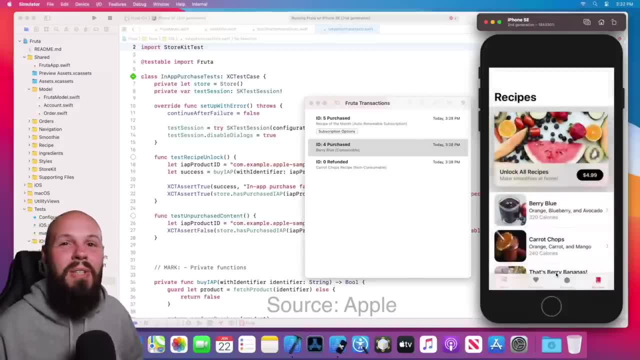 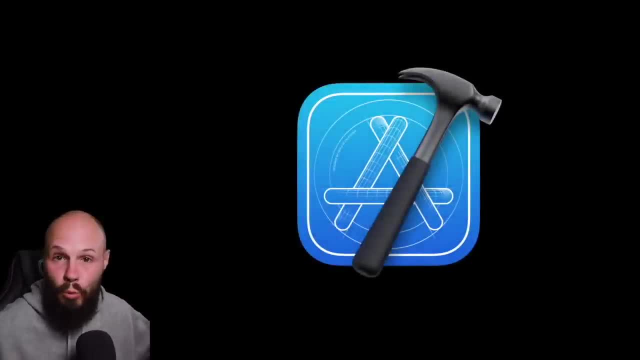 your tests. So that is much easier and much less of a headache than it used to be. All right, That's the highlights of Xcode 12.. Like I said, check out the link in the description for the actual release notes If you really want to dive in. it's very long and there's a lot of little stuff but this. 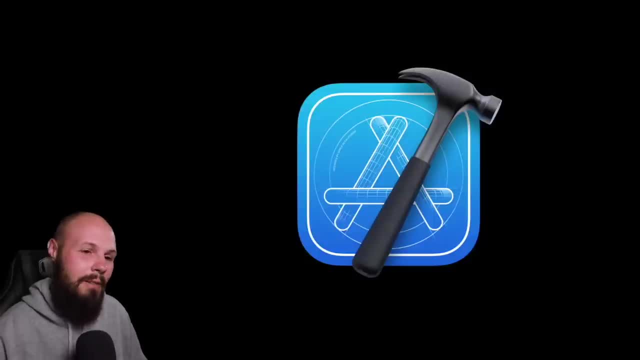 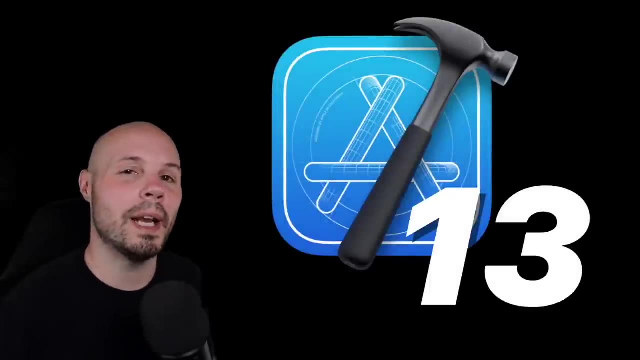 was the major highlights that I think a lot of people will use On a daily basis. All right, We'll see in the next video. Today we're talking about what's new in Xcode 13. We got some great improvements to co-completion. of them is now in Xcode. 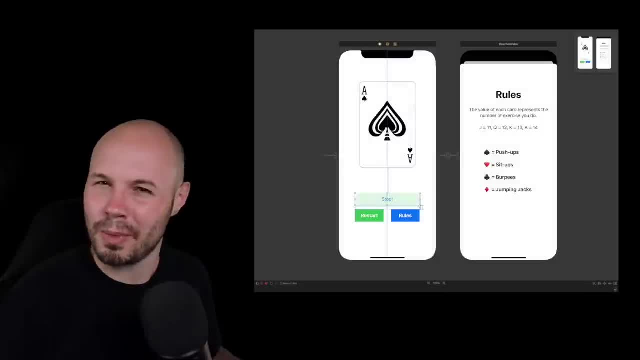 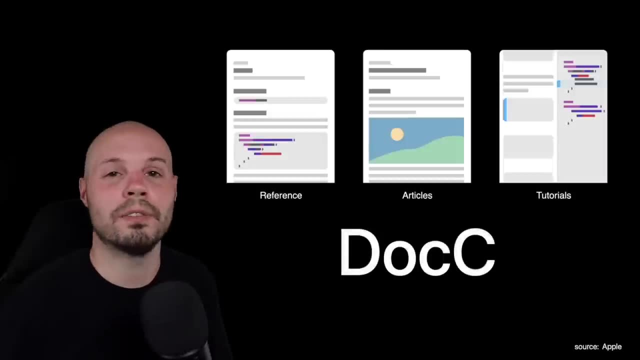 We have column breakpoints, some new additions to storyboards- remember those- and some nice design tweaks. And of course, we got Xcode cloud and then the documentation compiler, or doc C for short. Now Xcode cloud and doc C are completely different beasts all on their own 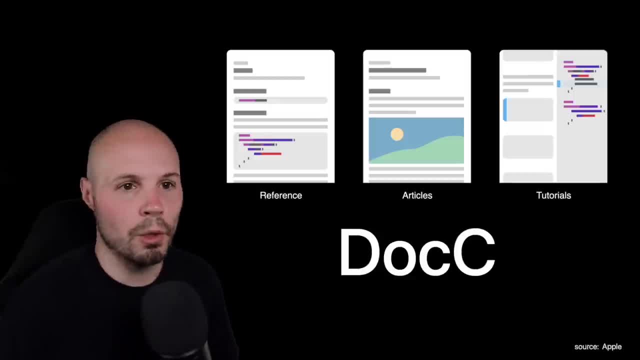 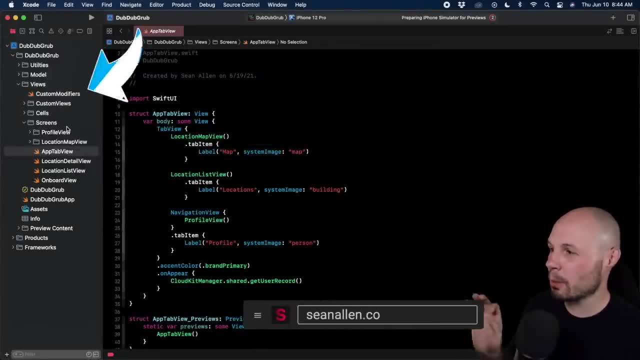 So, after I show you the day to day stuff, I'll give a brief overview on those two topics as well. Let's talk about some design tweaks first, cause that's quick and easy. So the first thing you'll notice- and I'm a real big fan of this- is the folders and 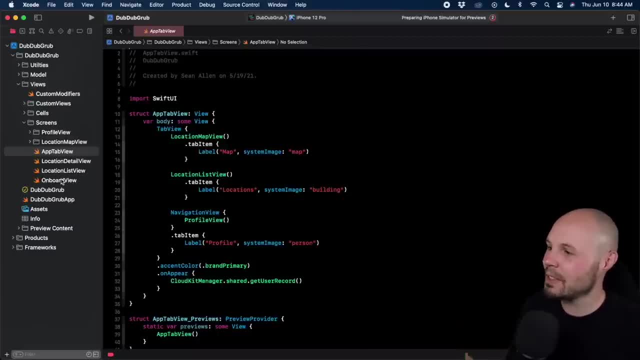 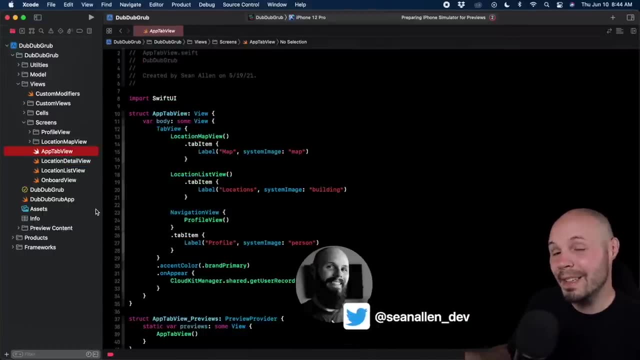 icons have a new look and feel. I like it. I think it's nice and clean. You may notice you don't have like the dot Swift file or dot whatever file. You can bring that back if you want. I like the cleanliness of it. 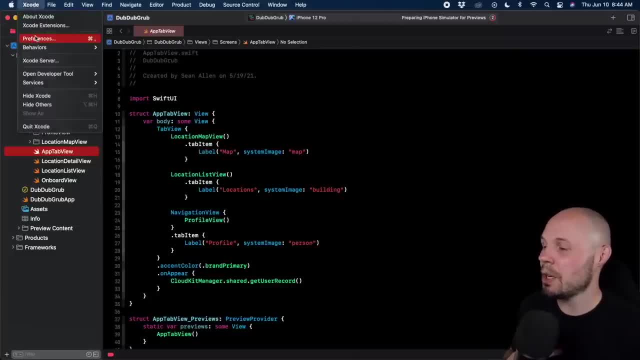 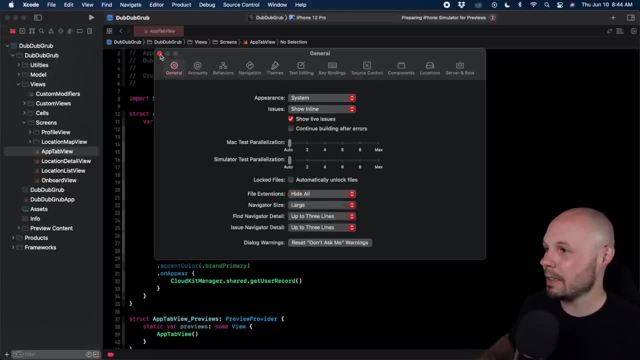 That's just me. But if you do want to bring back those file extensions, you go to Xcode preferences in general And then you'll see here file extensions hide all or show all. again, I'm going to keep mine hidden. I like the cleanness of it. 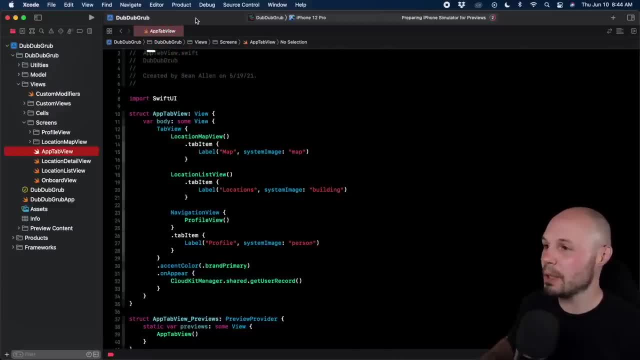 You notice, this top bar got a nice little addition too. You don't have to select your simulator or whatever right here. That is now moved over here. iPhone 12 pro right. This is where you can select that and then your schemes and all that stuff. 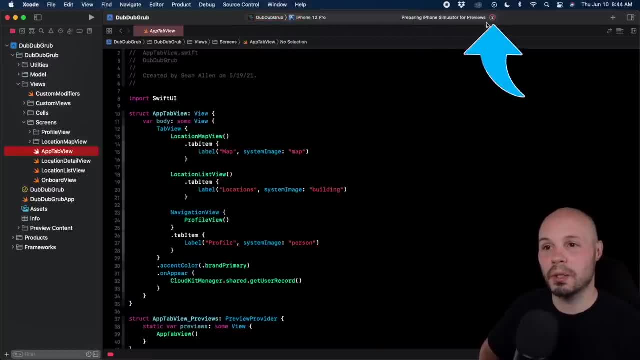 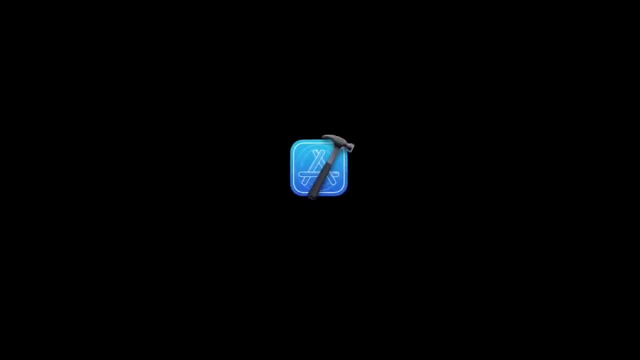 And then there is no more long horizontal loading bar. You get the circular spinner. So some nice little design tweaks that, in my opinion, really clean it up. I'm a fan. Okay, Let's talk about some of those auto-completion improvements I was talking about. 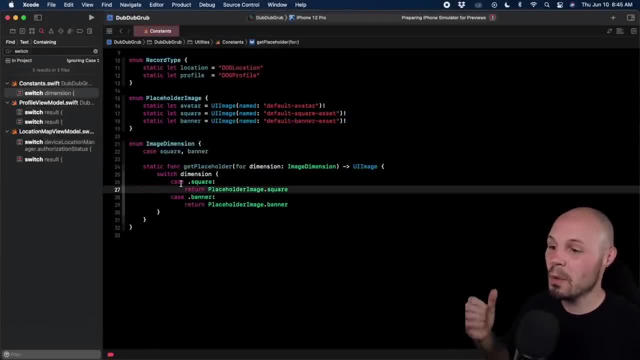 And my favorite- that's what we're going to start off with- is the switch statement. So in most cases, your switch statement will automatically fill for you, right? We're getting a placeholder image here, based on an image dimension which can be, you know. 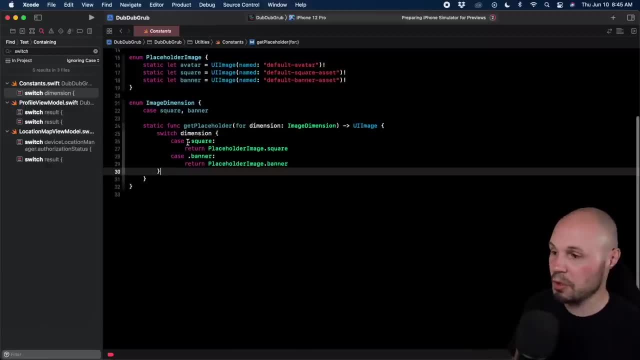 square or a banner. Well, I'm just going to retype this switch statement below so you can see it right. So I type a switch and then dimension, and you see in the auto-complete there's a little curly, brace version of it. 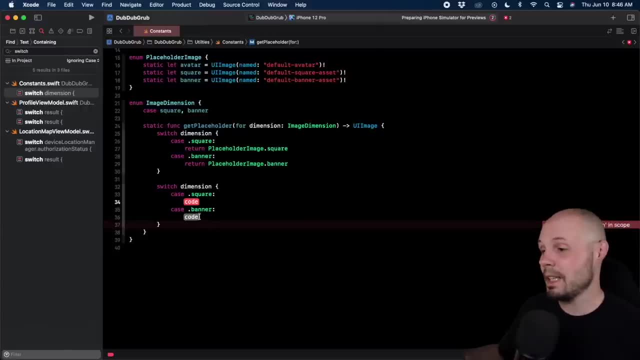 Well, if I hit that one, it's going to automatically fill in all of my cases. So that's nice. What I used to do is I would type that out and then- right, I wouldn't type this and I would you know. wait for Xcode to yell at me. 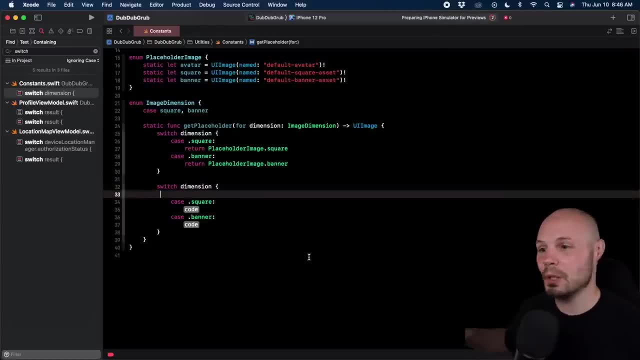 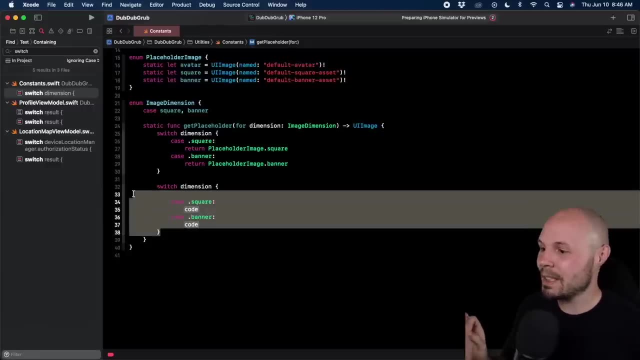 Switch must be exhaustive, Then I would click this and then I would fix that and it would fill in. So I love this because it saves me like two to three seconds every time I type a switch statement. Big fan here. However, it doesn't. I don't know if this is a beta one issue, and that's a quick disclaimer. 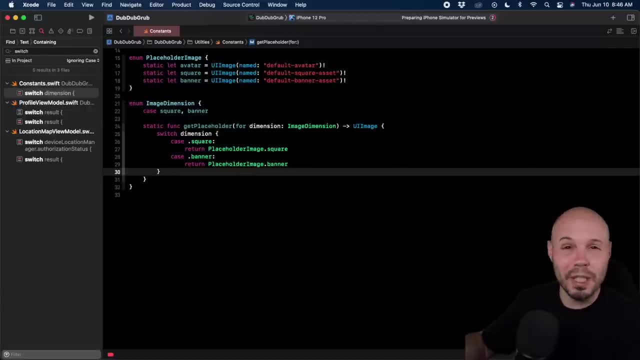 I should say is that I am in beta one, So things may not be working perfectly, Things may improve, things may get added, but we are in beta one. The most common use case for me on a switch statement is switching off a result. 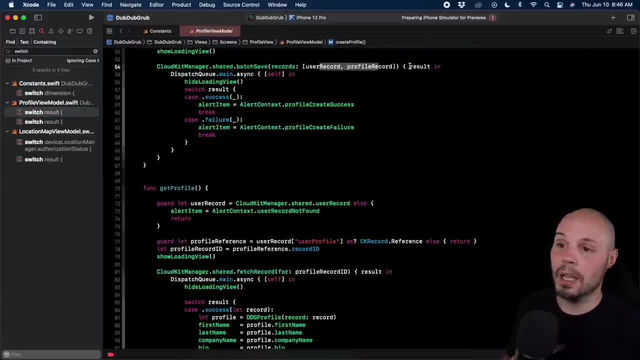 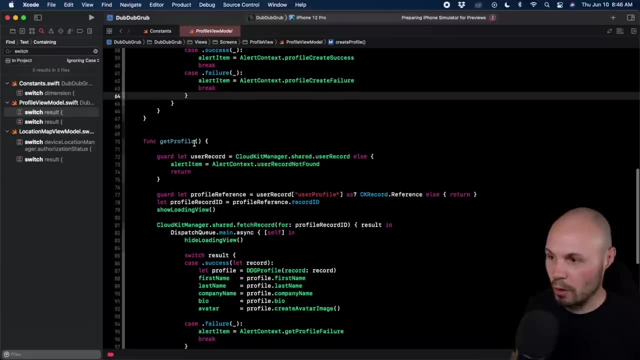 Right. So you see, here we are batch saving records. We get back a result with a network call right. You get success or failure, and then you act accordingly. Well, again, I don't know if this is beta one or I don't know if this is, you know. 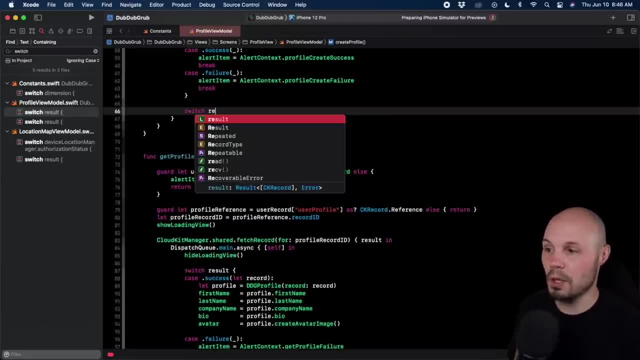 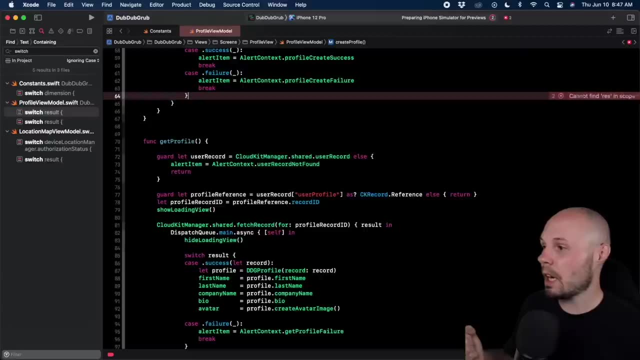 not part of the functionality, but here if I type a switch and then results like I don't get that auto-completion of the success and failure case, So just wanted to point that out. It seems to work great for your own enums that you've created, that you want to switch. 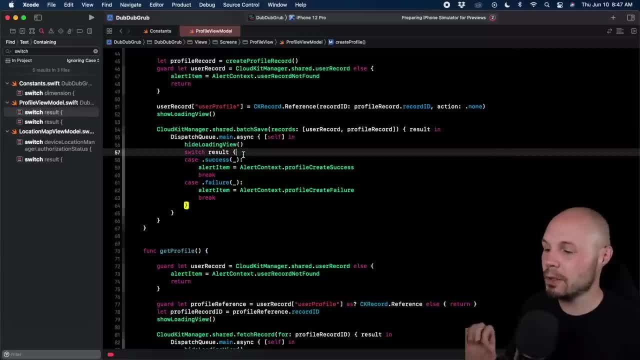 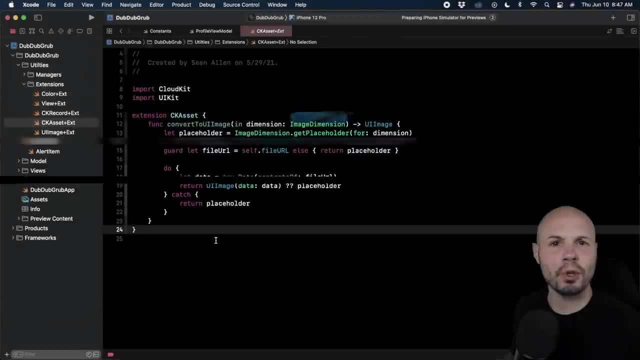 off of, But for something like the result case it's not quite working yet. Again, It could come in a future beta, but wanted to point that out. but overall, love this change. Another quality of life improvement is that Xcode will be able to recognize what frameworks 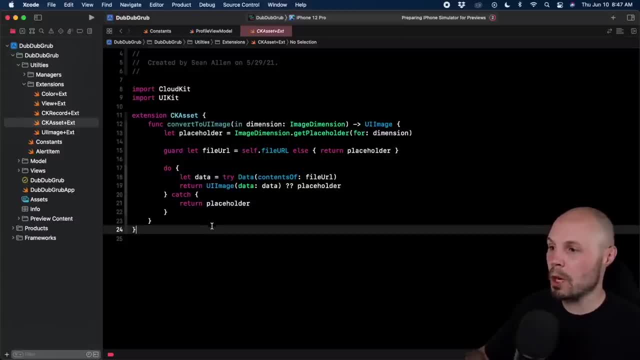 you need to import and then import them automatically. So here in the dub dub grub app we're converting a CK asset from cloud kit to a UI image- Cool. But you see, here we return a UI image here, so we need UI kit in our extension. 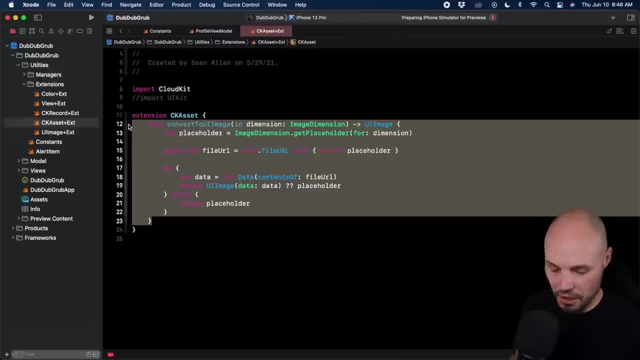 Okay, But let's comment this out. Pretend we don't have this. comment out the whole function. Cool, We don't have it. Now I'm going to retype that function here And you'll see it. It's going to pop in. 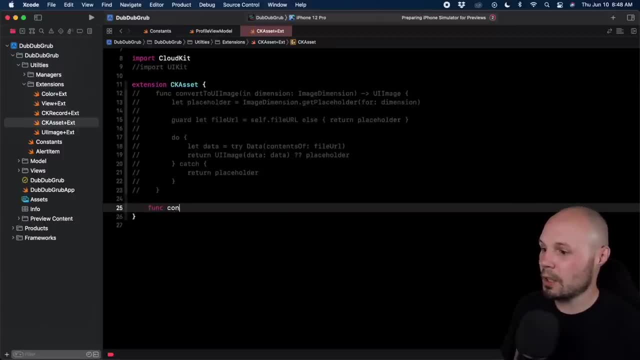 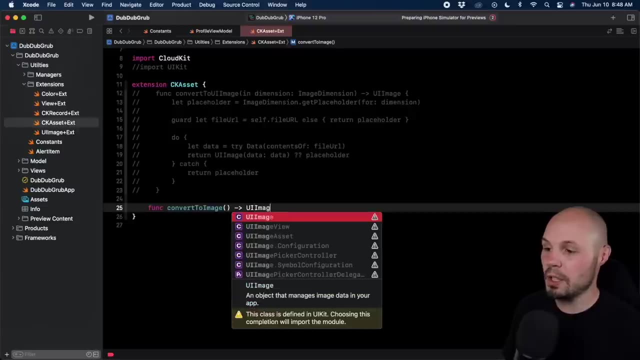 Let me scroll down so you can see the imports funk. convert to, I'm just say, image. I'm just going to type this out real quick, Not the full signature here, UI image. And you can see when I have the UI image autocomplete. there's a little warning. 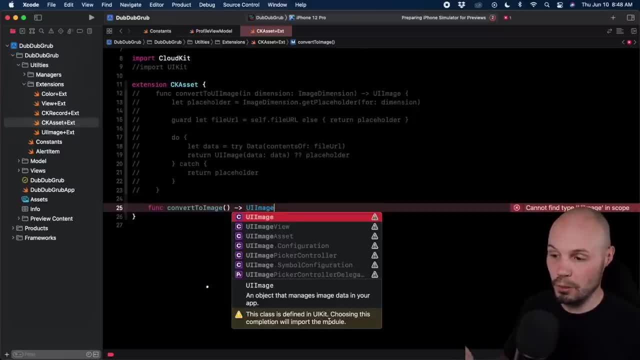 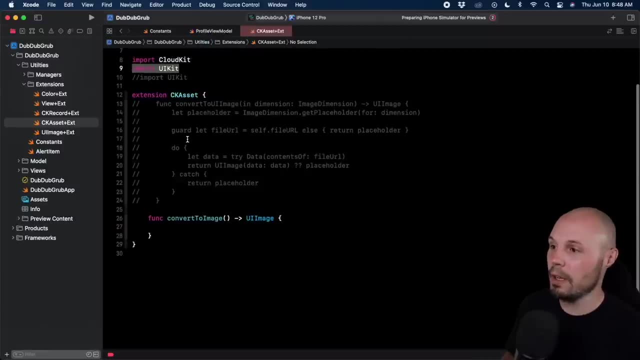 This class is defined in UI kit. Choosing this completion will import the module. Great, That's what I want. So if I hit return for the completion, you know, give me my curly braces- You'll notice UI kit got imported right away. 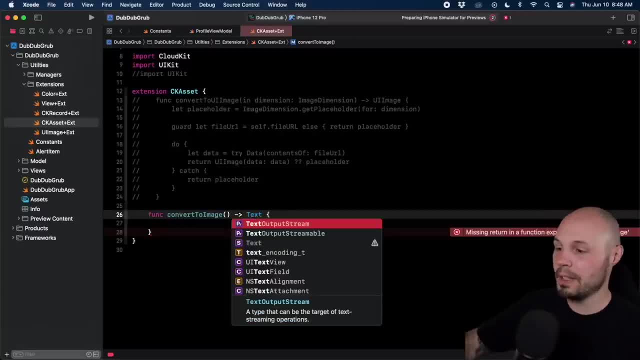 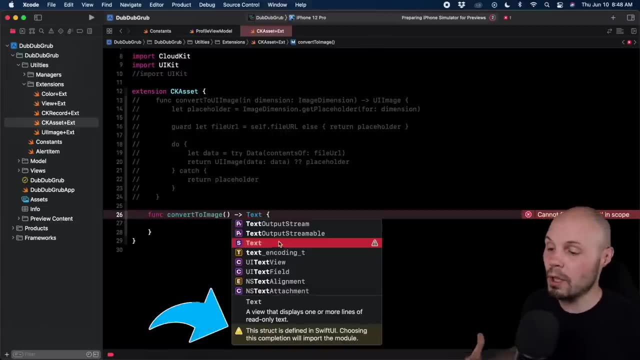 And if we change this UI image to you know text? of course I'm just experimenting, right that, don't worry about the function signature making sense, but we see, if I click this text right here, the Swift UI text is what I'm looking for. 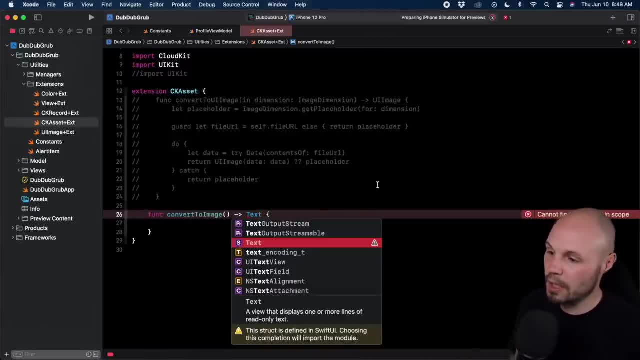 This struct is defined in Swift UI. choosing this completion will import the module. Great, That's what I want. And then now you see I have Swift UI up at the top. I think this is great because I know many times I have like tried to type something. 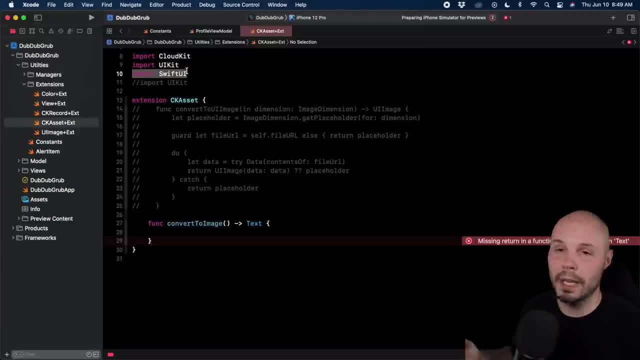 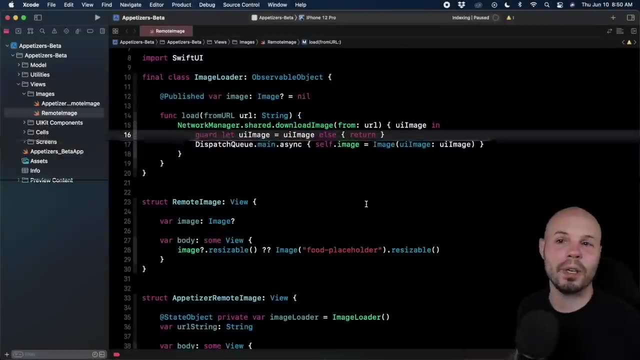 and I'm like, why don't I get the autocomplete? And it's like, oh, I forgot to import Swift UI or import UI kit, And here this does this for you, So big fan of that change. Next up, we have more auto-completion stuff with a guard leg. 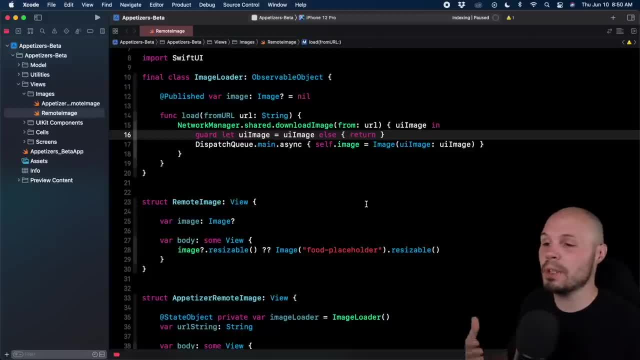 Let in if let right. when you're unwrapping optionals a lot of times, that will autocomplete now as well. So here's an example of a remote image loader. By the way, this is getting replaced by async image and Swift UI. super pumped about that. 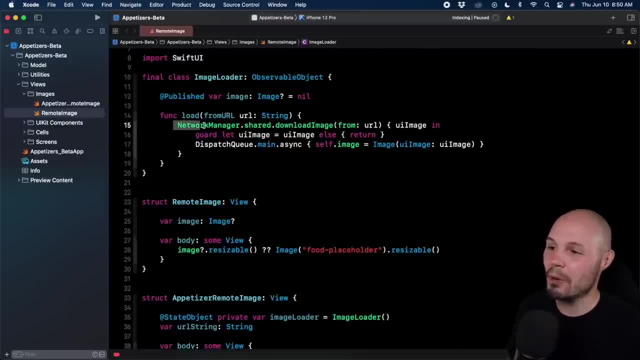 So all this code will be gone eventually. But we're using this example here, right where we're making network manager call to download the image, We get back an optional UI image. So before we use that UI image, right, we have to basically make sure we have it. 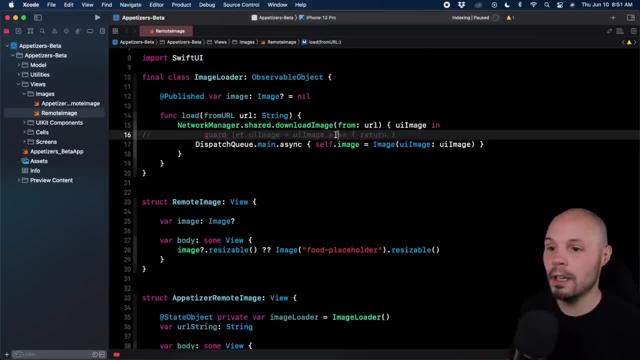 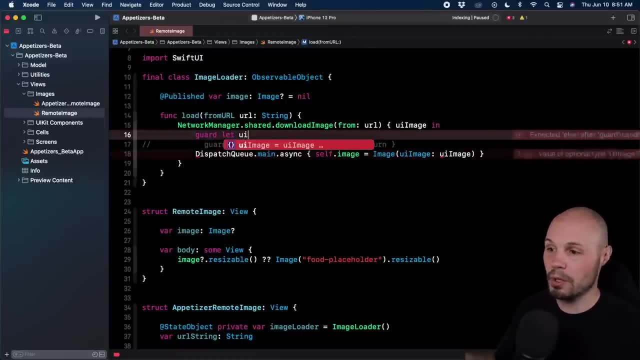 So we unwrap the optional. Well, if I just comment out this line here and you'll see, when I type guard, let UI image- right, UI image- I get the autocomplete for the rest of it right before that didn't happen, right. 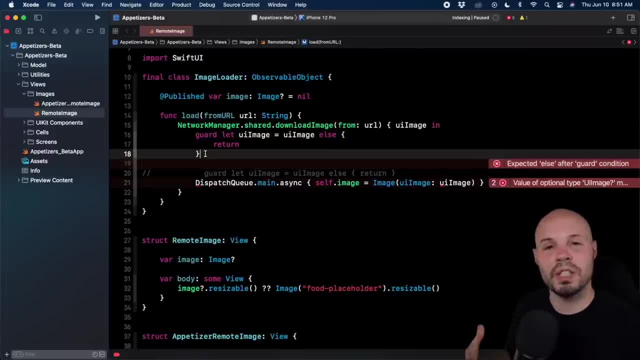 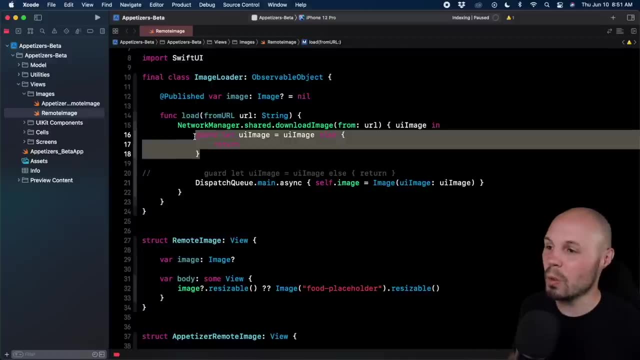 Hit return. Now I get the autocomplete for my guard statement. Now, similar to the switch statement examples I showed, if the example is simple like this, there's only one- works great. If it's a little more complex, it doesn't seem to be working that great. 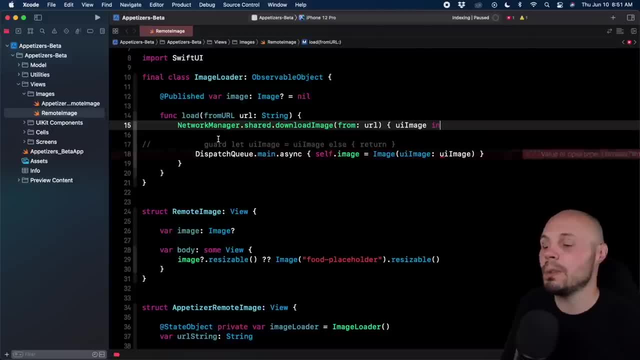 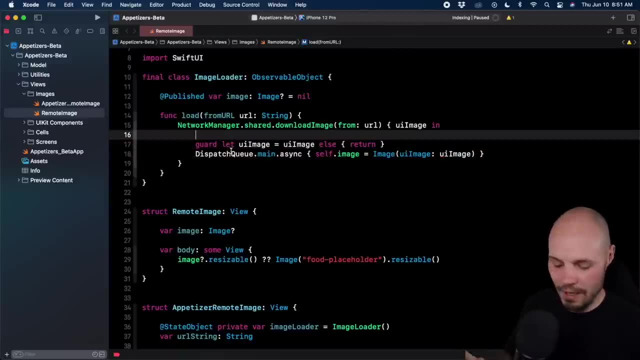 Again, I may be trying to do more than it's intended to do or it could be a beta one thing, But I just wanted to point that out. And of course you can have more complex guard let statements, But again, for the simple ones, it works great. 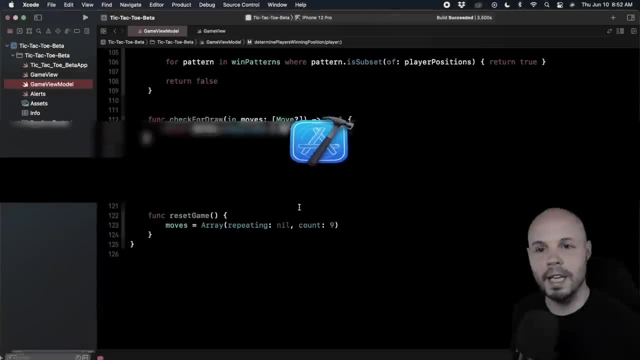 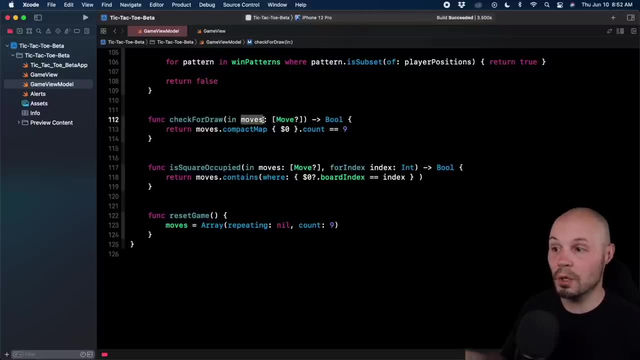 And again a welcome addition. And for the last of the autocompletion improvements, we have the singular version of for loops. So you see, here I pass in an array called moves. So if I do for move in, moves right, normally you have to type all that out. 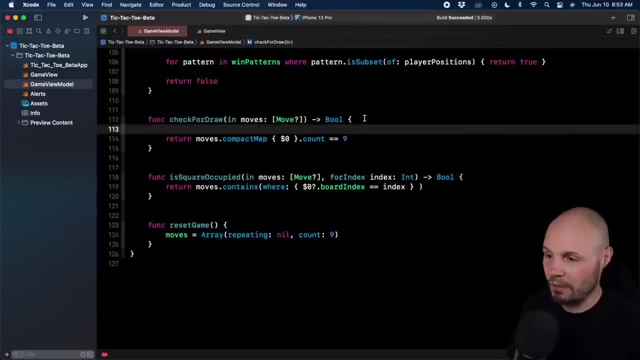 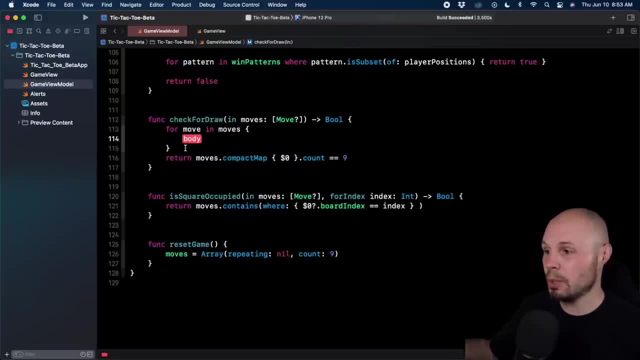 Well, it will recognize the singular version and autocomplete that for you, right. So if I did for move, right, you see, for move in, moves, there you go, it knows, and it completes my for loop. And I saw Paul Hudson playing around with this and thought it was pretty cool. 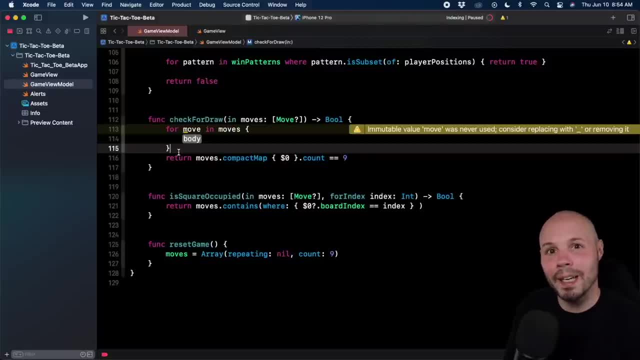 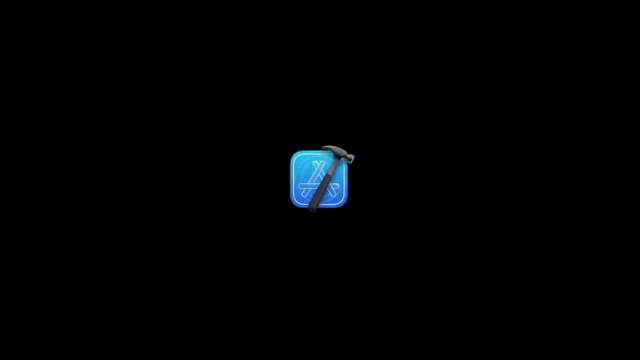 It'll show something like for goose in geese right. It'll recognize that goose is the singular version of geese, So in some cases it is able to recognize that and I thought that was pretty cool. Next, let's talk about column breakpoints, right. 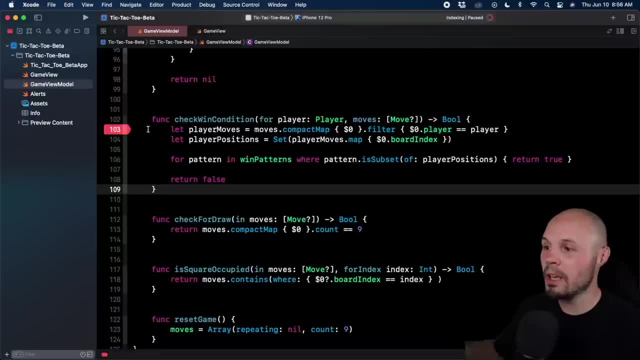 So we're used to the line breakpoint, right? You see, I just put it on 103, it will stop. you know, before or after it runs this line wherever you put it right, But it's the whole line. Well, you'll notice, especially when you're using some higher order functions like compact. 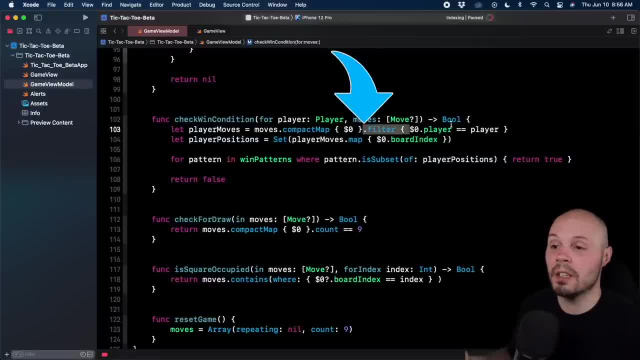 map, or map or even combine where you can like, chain this stuff together. well, you know, just the line isn't. we're not gonna be able to debug that, Because we wanna be able to stop this, you know, somewhere mid chain. 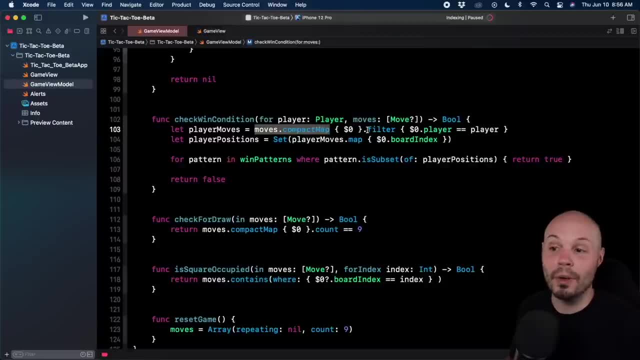 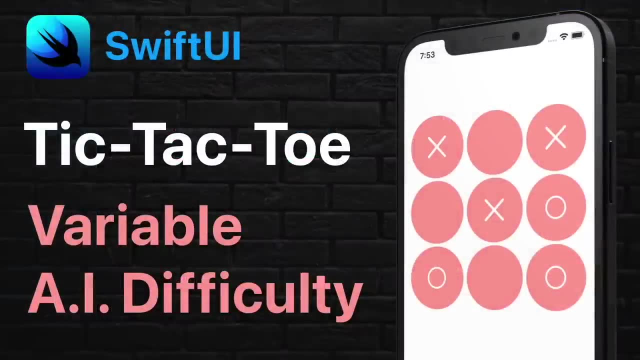 So to do that right, let's say movescompactmap. before I filter that, I want to make sure my movescompactmap is what I'm expecting. And, by the way, this is from my tic-tac-toe tutorial, where I basically take all the moves. 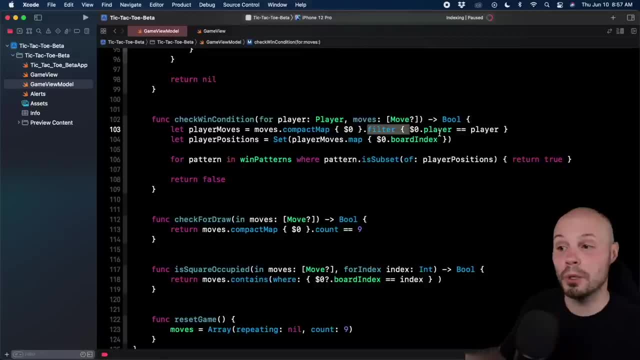 get rid of all the nils and we're filtering, you know, all the human players, or all the computer players which we're passing in here. So that's what's going on here. That way I can see what moves the human has made, check for the wind conditions, all that. 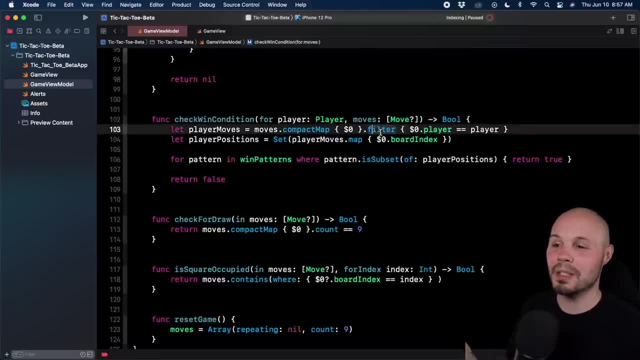 stuff. So that's some semblance of what's going on with this code, But let's talk about this column breakpoint. So if I right click filter, go to show code actions and then set column breakpoint, And then you see this little vertical breakpoint, right? 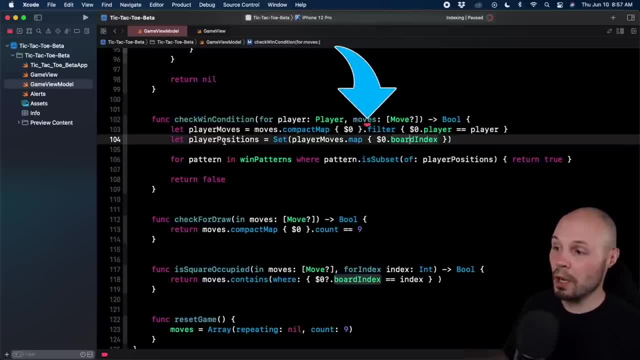 I'll click off filter so you can see it. So now what's gonna happen when I run my code? it's gonna run this portion of the code and then break right here before it does the filter. So let's test that. And actually, so I have some moves in here- I'm gonna turn the breakpoint off just by. 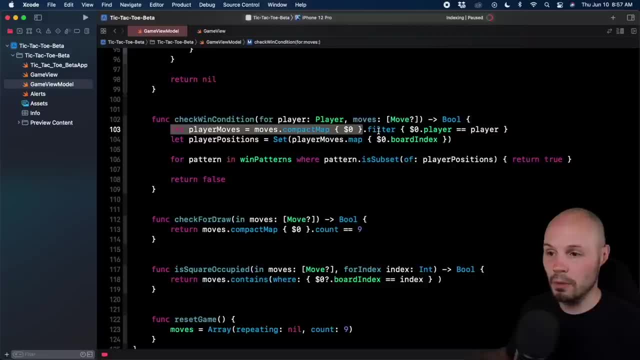 clicking it And, by the way, to delete it, you can just drag it off. So, okay, we won't add the breakpoint now. Let's run the program. I'm gonna, I'm gonna make some moves in my tic tac toe game. 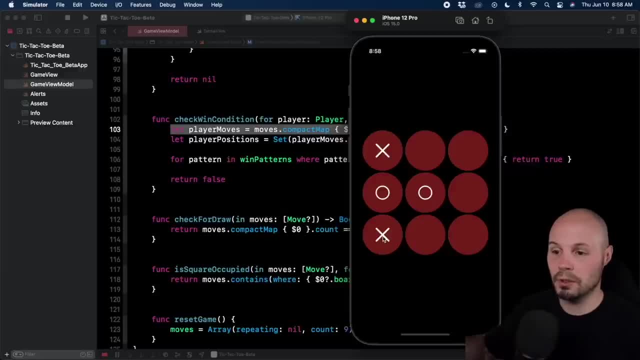 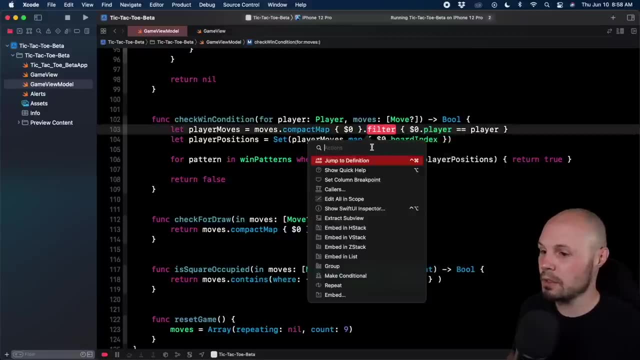 So some moves are in there. Okay, now the computer goes, I go, computer goes. okay, we got moves. So go back to the Xcode. Now put the breakpoint on the filter. So right click show code actions, column breakpoint. 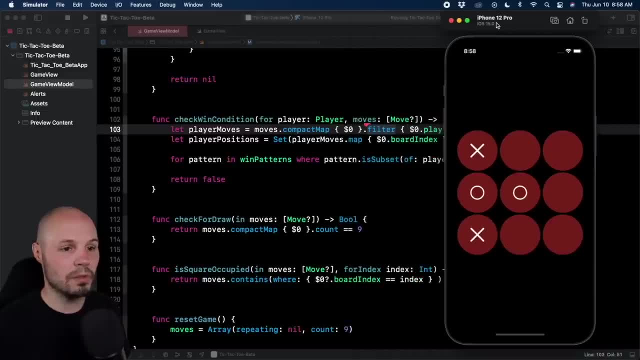 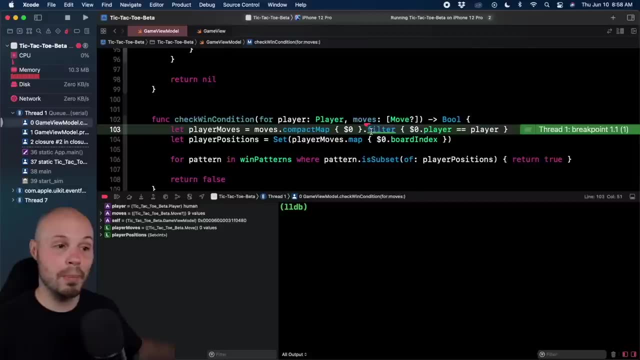 There we go, And then back to the simulator. here we'll move this over. Now I'm gonna make a move where I block circle right there. Okay, the breakpoint broke right there, So I have moves dot compact map. that has happened, but the filter hasn't happened yet. 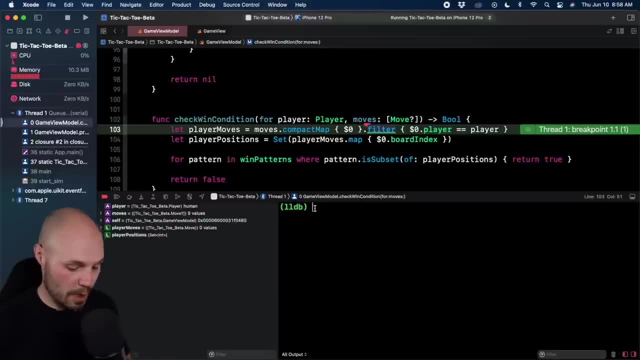 So say, I had a bug And I wanted to check my moves dot compact map So I can do PO moves dot compact map. dollar sign: zero hit return, Here we go. So this prints out my moves here So I can see before I filtered right, I've gotten rid of all the nils. 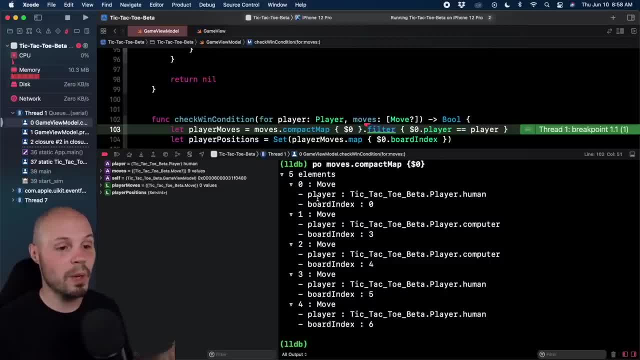 That's what compact map does. by the way, it gets rid of all the nils. So I'm left with just my moves, And you can see I have like human moves: human move, human move, computer move, computer move. 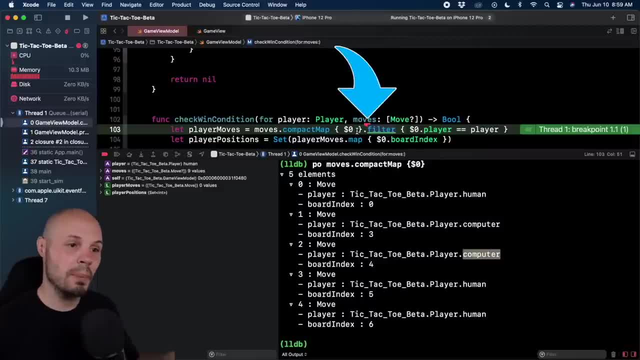 So this is before I filter it. So again, column breakpoint stops a line if you have something chained so you can break before something happens in the chain and then inspect, debug, do what you gotta do. So column breakpoints, again another very welcomed addition. 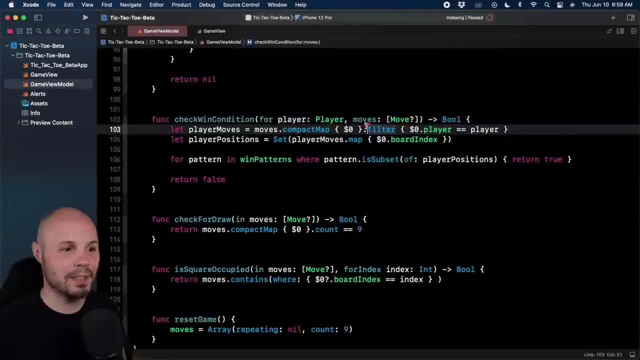 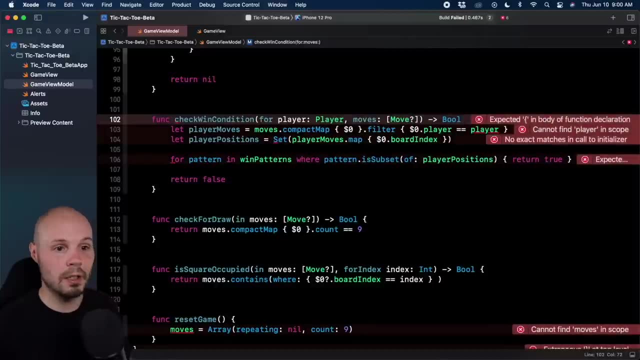 All right. next we have some error. cleanliness- All right. so let me get rid of that breakpoint. I don't know. let's break this right. Let's get rid of a curly brace here. That's gonna send everything into a tizzy. 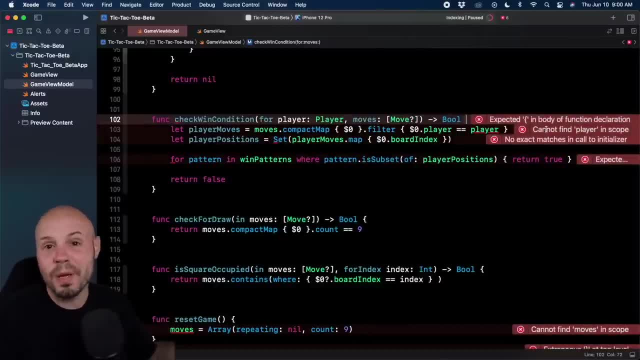 Okay, look at all these errors. Now you see how these are all in your face. Sometimes you may want that, But this also applies to warnings as well. So if you don't want all this clutter, there's a way to minimize these. 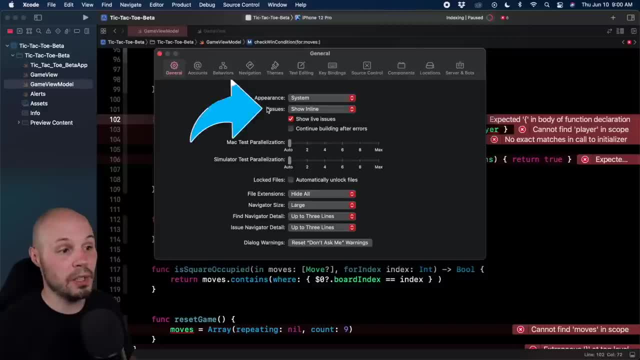 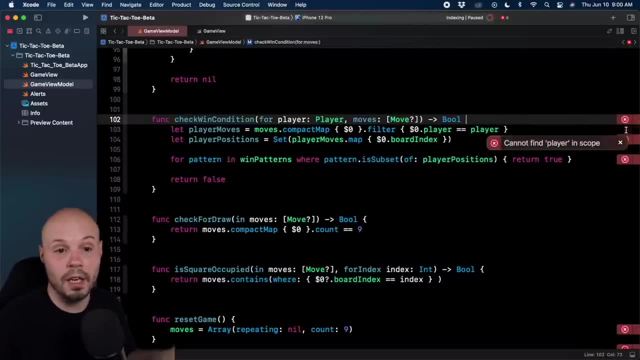 So if you go to Xcode Preferences And then you see issues, instead of show inline, hit show minimized and you see they all minimize over to the right Now you can still see them right. You click on it. you can still see what the issue is. 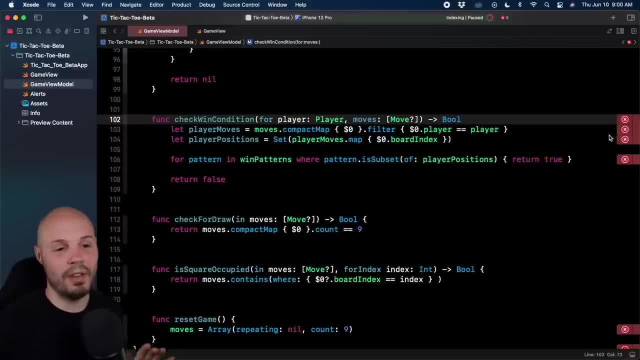 There you go, But it is just not so in your face. So this is obviously a personal preference thing. If you want your errors and warnings to be in your face, great, leave it, don't do anything. If you want them to be minimized, now you have the option. 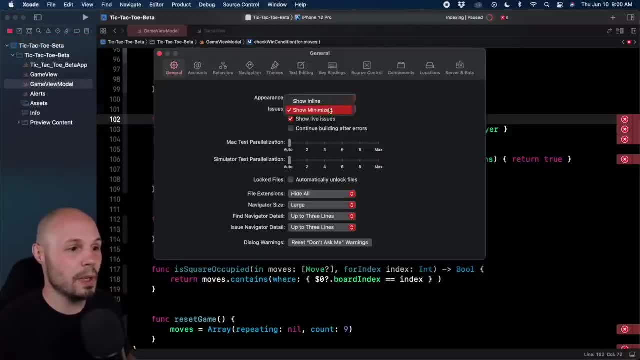 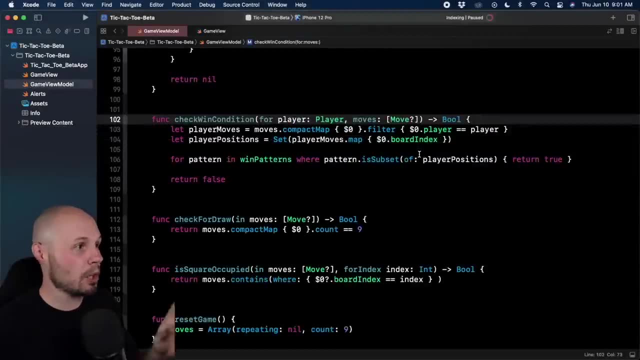 So that's cool. And again, Xcode Preferences. Instead of show minimized, show inline. and there you go. Next up, Vim is now in Xcode. I'll show you how to enable that. So Xcode Preferences. 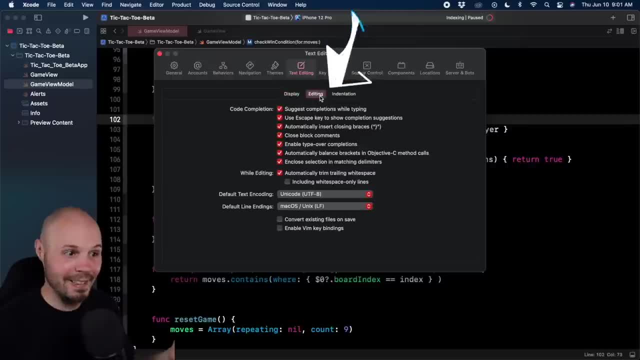 Text editing. It's a little buried Editing- And then enable Vim key bindings And then you'll notice on the bottom you see kind of the little shortcuts. you get down there to teach you how to use it. Now, if you're not familiar with Vim, Vim is like a completely different way to navigate. 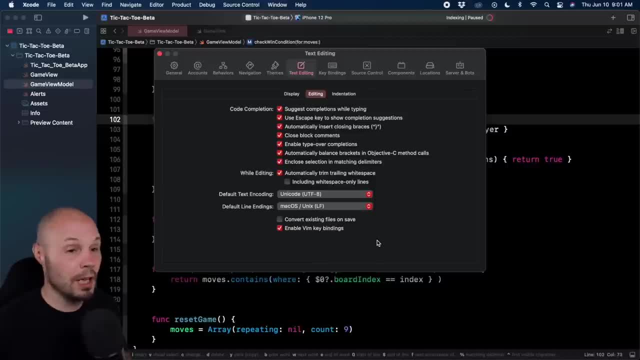 via just keyboard keystrokes. Very steep learning curve. I tried it once a couple years ago. gave up very quickly. So I'm not a Vim user, But I know many developers swear by it and they say: once you learn it, you can never. 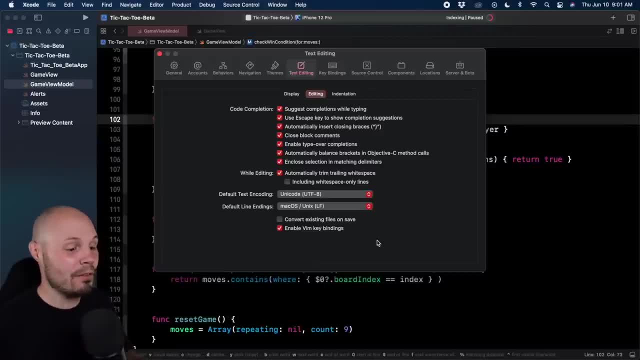 go back. I'll take your word for it. But anyway, if you are a Vim person, that is how you enable it. Now you can use Vim in Xcode. A little bit of a warning- from what I've seen on Twitter anyway, is that it's not 100% there. 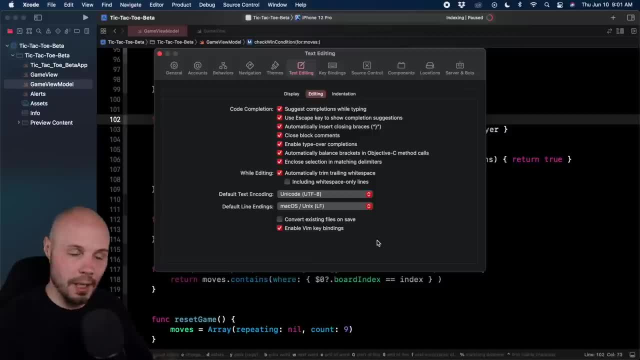 Like maybe 90% of the functionality is there And I don't know if that's just again beta one. maybe it'll improve over the betas, Or maybe this is something. in every Xcode release we'll see a release note that says: 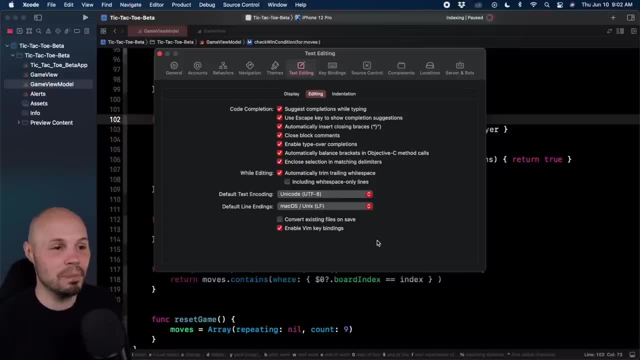 Vim improvements. Added this to Vim Official launch of it. if you will, So again, if you're a Vim user now, you can use that in Xcode by again Xcode preferences text editing. editing. enable Vim key bindings. 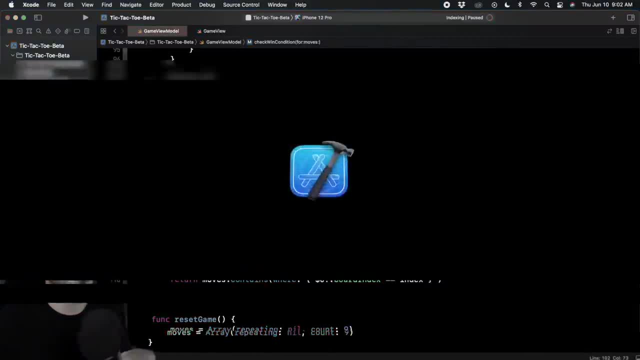 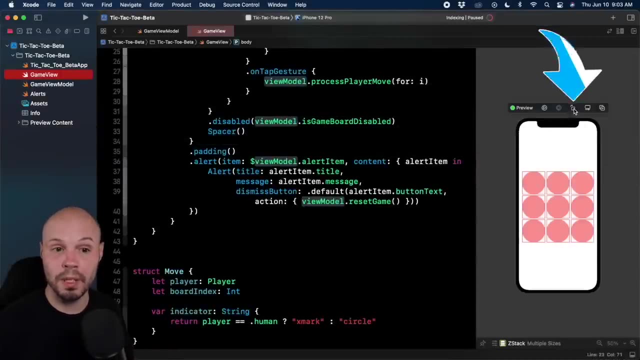 I am going to turn those off because that is not for me. Now some quick updates to SwiftUI previews. We got landscape mode in previews. you can tap this little button right there and you can see what your app looks like in landscape. And we did not account for landscape in the tic tac toe app, obviously, but that's a nice. 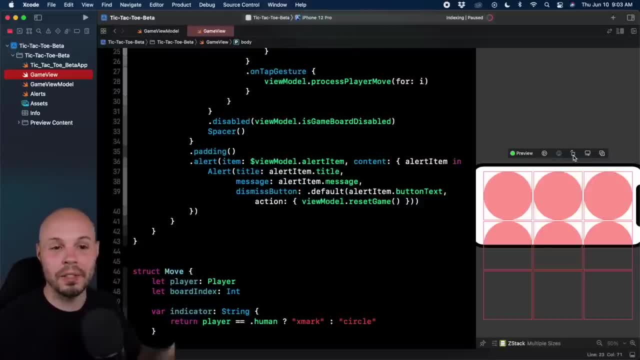 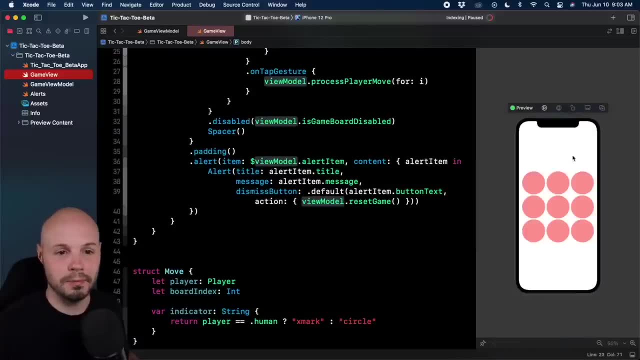 way to test it very quickly. And then you click this back. you can see it's going to keep rotating it to the right. See, now we're upside down. the notch is on the bottom. click it two more times. There's probably a quicker way to do that, but you know that's what we're doing, right? 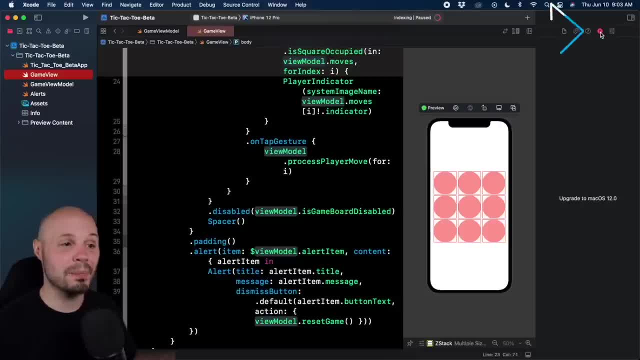 now. And then, lastly, on the right pane, you'll see we have access to the accessibility indicator right now, But you can see here: upgrade to Mac OS 12.. I can't upgrade to Mac OS 12 on my main machine. I can't take that risk. 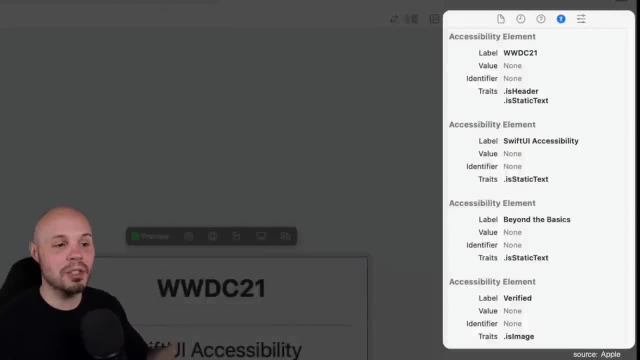 But I will try to get a screenshot of this on the video so you can see it. But essentially it's a nice way to inspect all of your elements to see what you have and what you're missing for accessibility. So it's a nice quick look to get your act together in supporting accessibility on this. 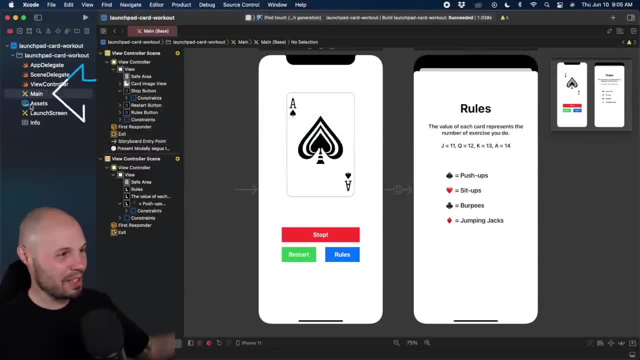 Moving on to the storyboard improvements, remember those right. First off, you see the nice little storyboard icon over there. Again, all the icons changed pretty cool Down here at the bottom in the canvas. you see we can get iPhone 11 and you can see we. 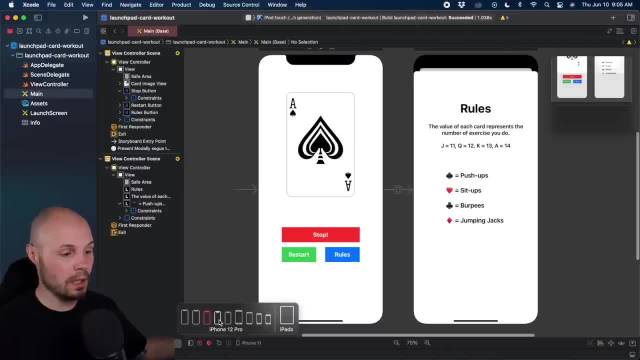 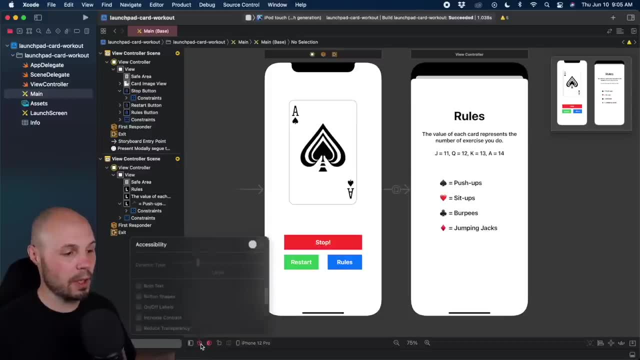 can go to the iPads, iPhones- we can switch back iPhone 12 Pro, So nice little UI there to switch phones very quickly. And then we also have an accessibility pane here right Where we can click this and view dynamic type. 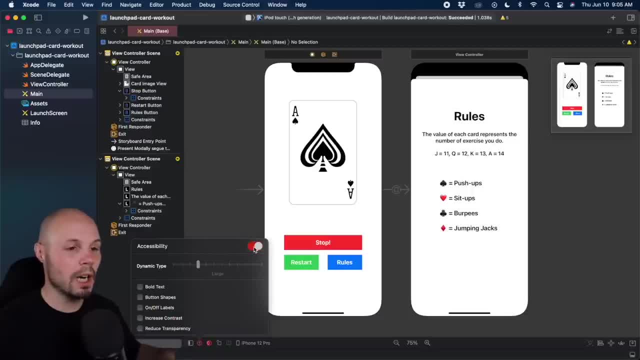 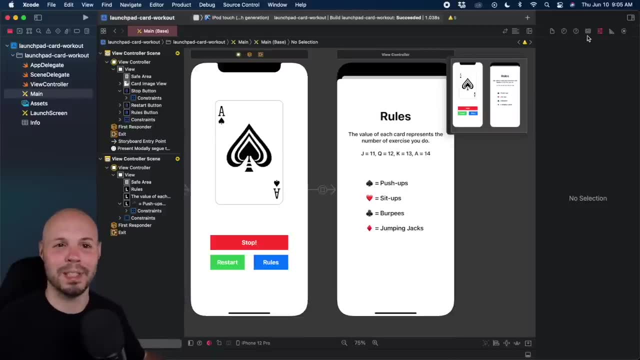 Okay, so our storyboard doesn't quite have that, so let's change that real quick Because, again, this is my super beginner app. We're teaching them how to build an app. we're not even touching dynamic type and accessibility, yet. This is the very first steps. 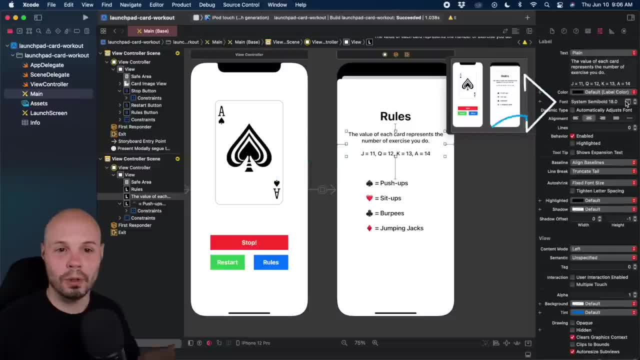 So let's go to our rules here. change the label here, right where we're hard coding the font. So let's change the text to: instead of system let's do body Should be all we need for right now. So get rid of this for the show. 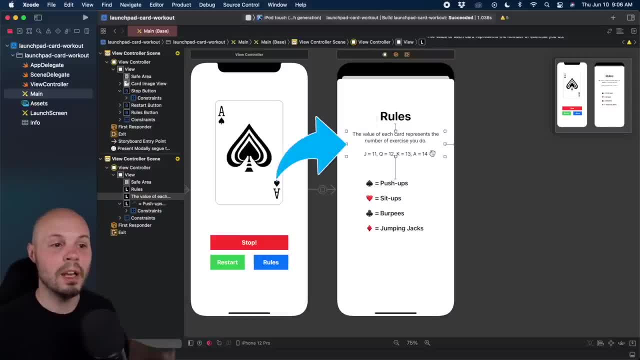 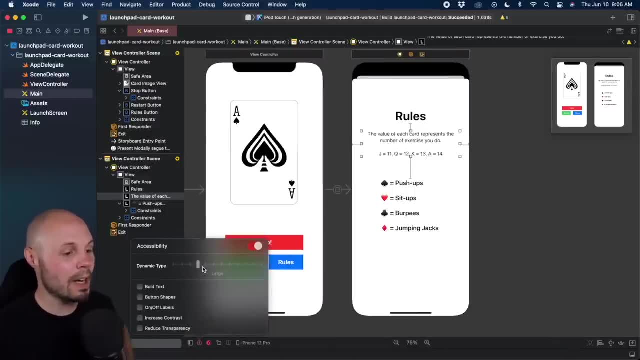 So basically what you're seeing here in the square, the rules- The value of each card represents. that is now body. So that will now support dynamic type. But what you can test now in the accessibility pane here, turn it on Now as I drag my dynamic type. watch the rules thing, right. 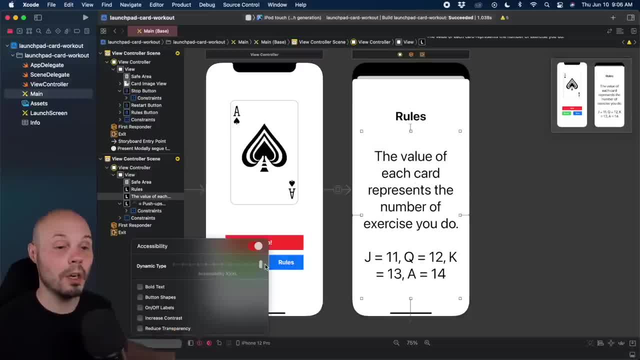 So you can see extra large, XXL, XXL. okay, obviously we're not supporting dynamic type. very well, It completely messes up the whole screen, but you can quickly see how this works again: Super, extra small. What does your UI look like? 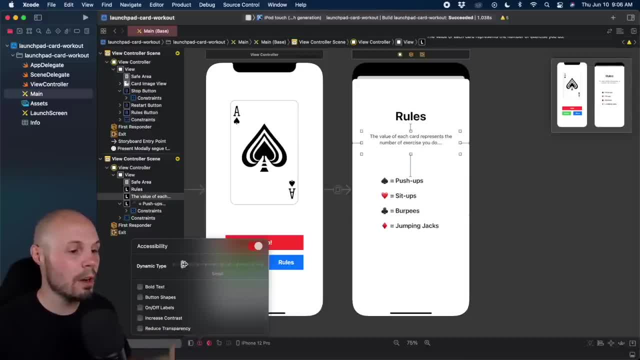 And you can just drag the whole way. So that's really cool to test your storyboard apps for accessibility. And there's other accessibility things, right, Like bold text. There you go Button shapes. I'll move this over here. You can see it has the underline on the button. 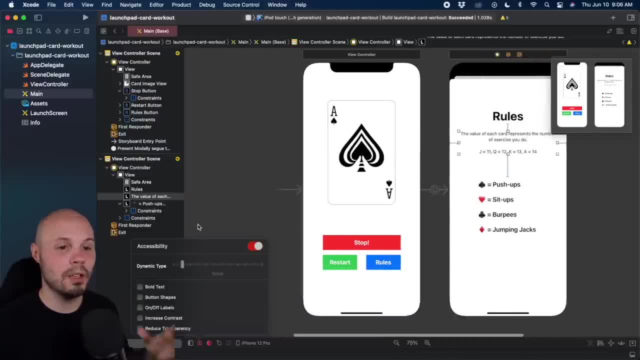 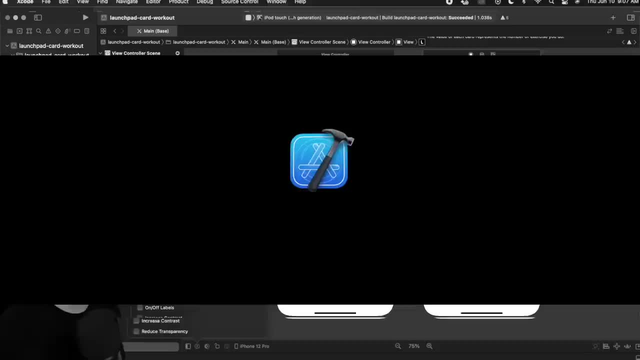 On off label. I don't think you can see the other ones, but anyway, you can just test your accessibility right in storyboard, And a good one is the dynamic type. Seeing that in real time, Very nice. Now let's talk about buttons on storyboard, because buttons got completely revamped in 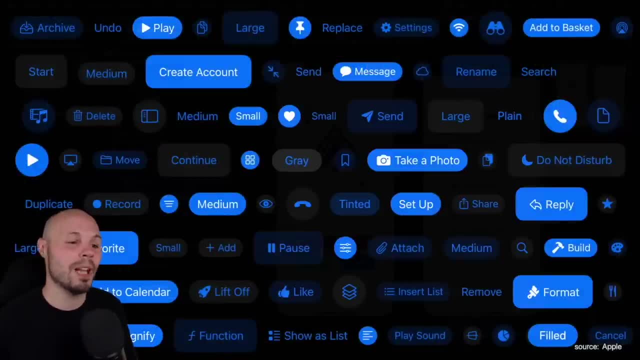 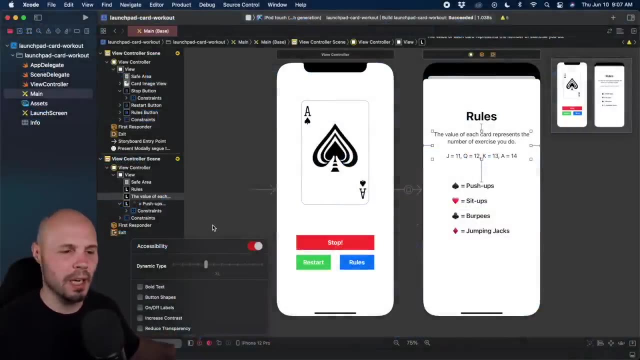 a very good way in my opinion, because I've written many a button subclass to try to get that default Apple look. Those can all go away now because they're built right into the new You I button API in button API in Swift. That's also built into storyboard. 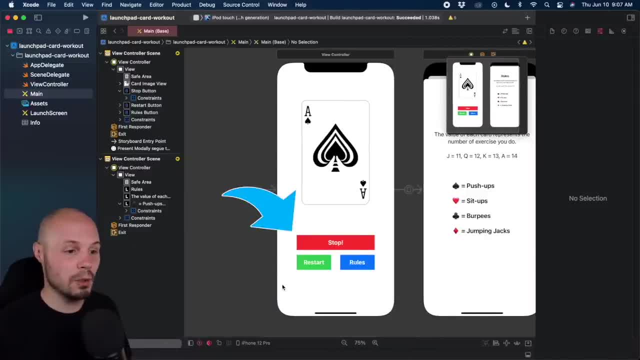 So let's take this stop button. Let me get my right pane out here, So we'll click on the stop button and you can see on the right pane over here all this stuff. I'm going to actually make this look like a default button, because before you had to. 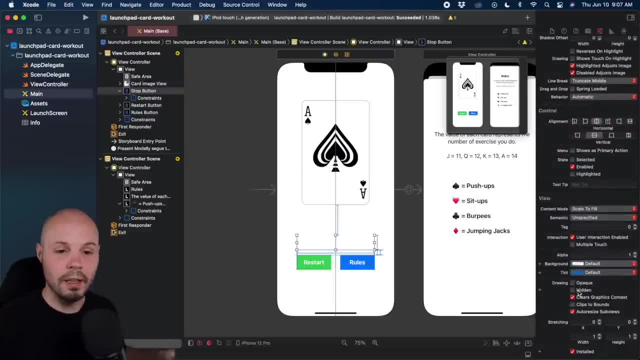 change the background color right to the color you want it. So let's get rid of that and let's go up and make the text color default. right, I want to. I want this to look like just the default button. There we go. 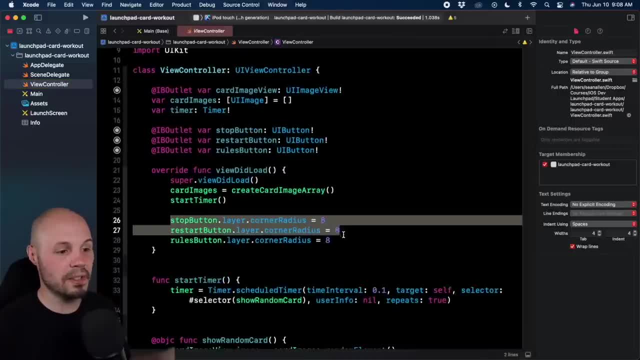 And real quick. you can see in code here on the UI button I had to make the corner radius eight to get the rounded corners right. I had to do a lot to get that look. So back to the storyboard. there's a new property here in the inspector called style and you 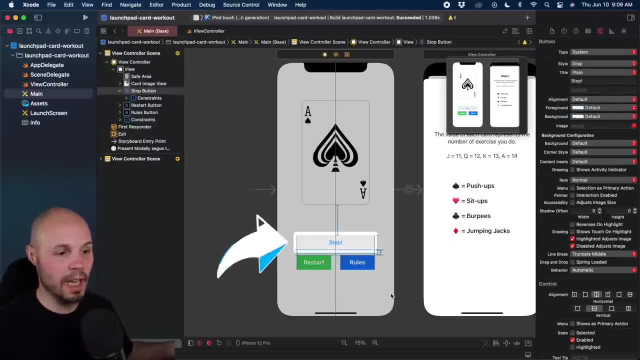 see I can do plain. Well, plain will look like that gray and you see, you get that, that grayed out style, See on the button there. and then, okay, back to the button. This is the one I like and I think I'm going to use in a lot of my apps. is this tinted? 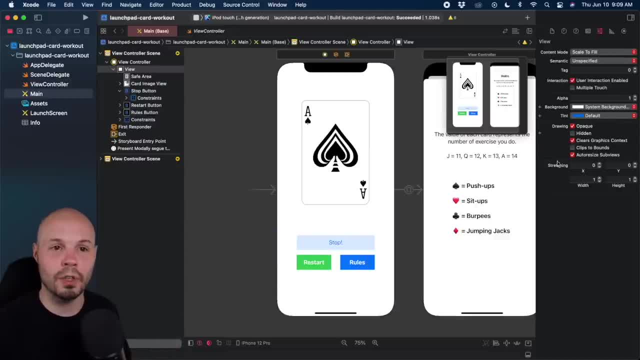 one right. So you get that tinted with the dark color. That's good for visually impaired people, because sometimes two different colors don't contrast nicely. but this is guarantees your contrast ratio pretty much. So back to the button and then you can do the classic Apple button. 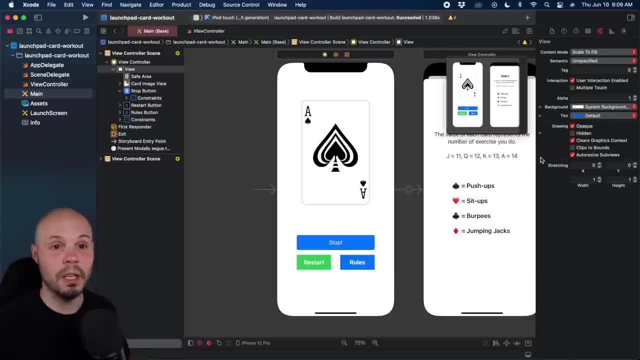 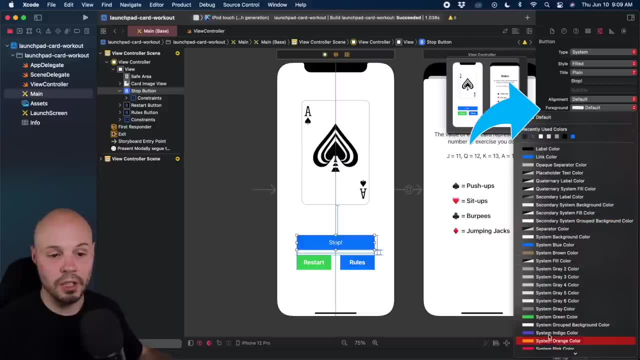 Which is this is the button that I always kind of built myself, was this filled button? And then also you can see there's other things you can do. So of course that's the color right. So foreground and background, you can change the colors. we'll make it green. 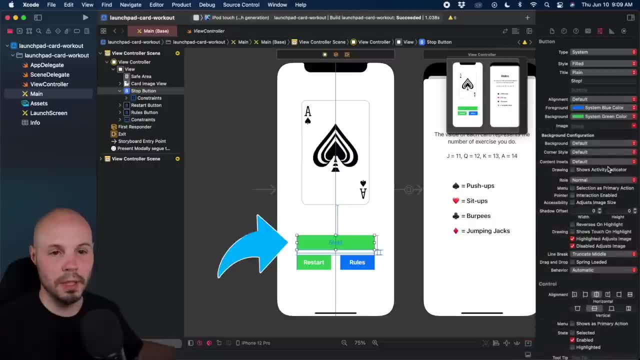 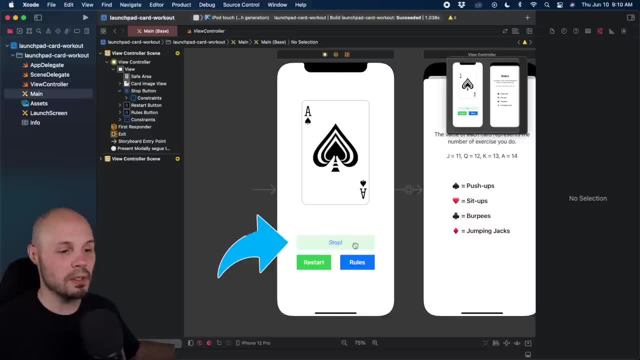 So green and white and then the foreground. we'll make blue just for example purposes, And then now that's the filled. right Now, if I go to tinted, you can see we get the tinted green with the blue. So you can customize this a bit on your own. but the last thing I'm going to show you is: 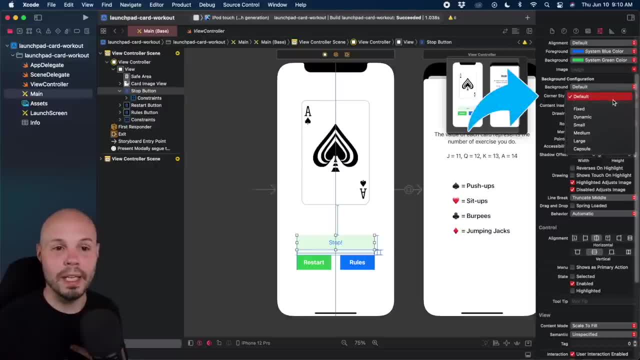 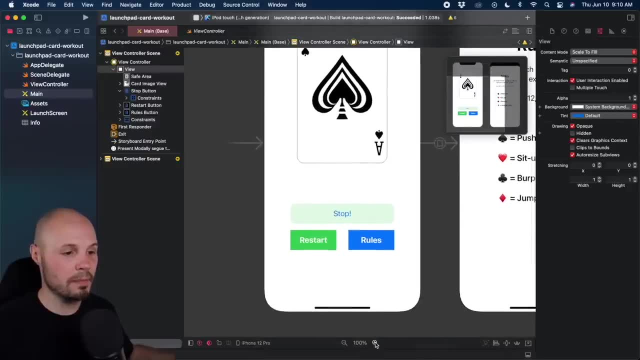 the corner style. Remember I said I had to do corner radius in code. Now we get. So basically small, medium, large corner radius, we'll do large corner radius. I'll zoom in here so you can like really see that. So there, that's large corner radius. 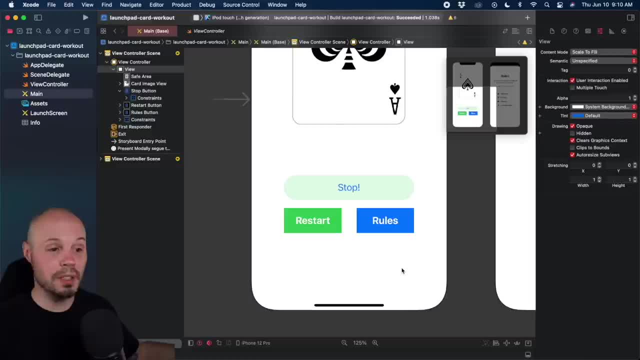 And then if I click on the button capsule again, this is another very common style that you used to have to write some code to get. Now you can just get that out right away. So the point is here: UI button got a complete overhaul and is built into storyboard to where 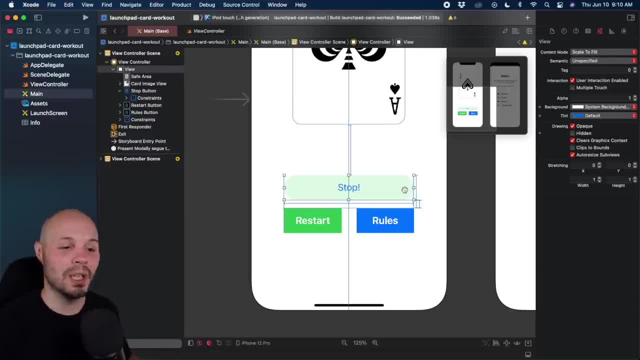 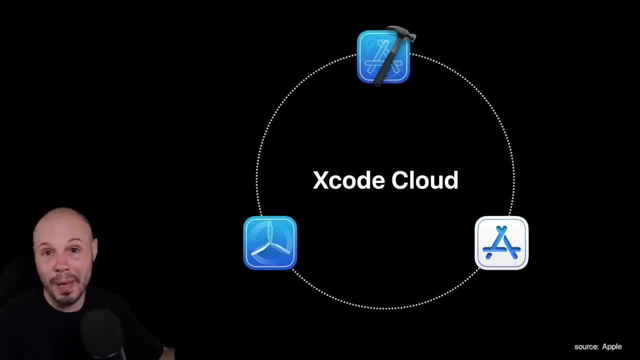 you can just, you know, click some buttons over here on the right to get your button to look how you want. Now let's talk about Xcode cloud. Well, first of all, Xcode cloud. It does require a beta invite, which I don't have access to, but even if I did have access, 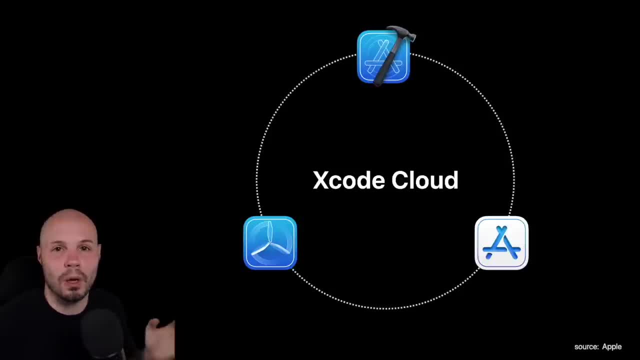 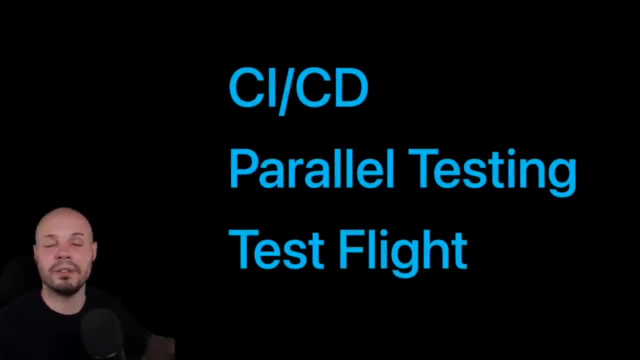 to it. it would be very hard to demonstrate because Xcode cloud is very focused on teams, Things like continuous integration, continuous deployment. You can build and run tests up on Xcode cloud on all kinds of various devices, all at the same time. 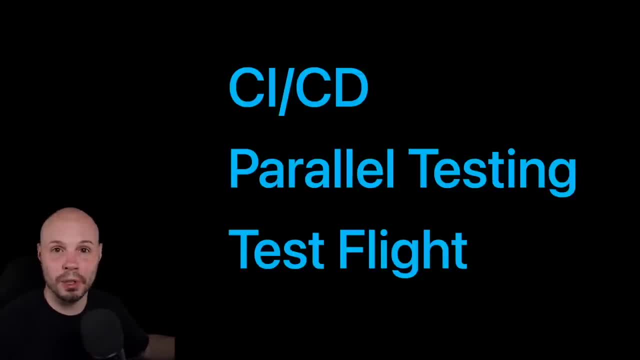 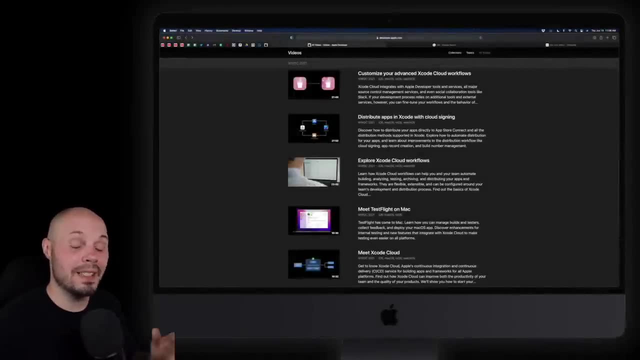 And then, once they all pass, you can automatically push the test flight to go out to all your beta testers. So if you want to dive deeper into this, I'll put some links to the WWDC talks- all about this. There's a few of them. 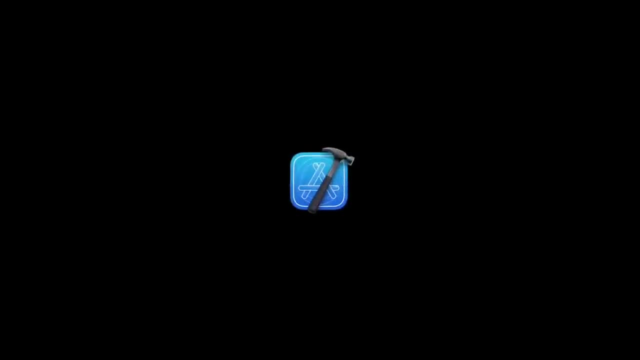 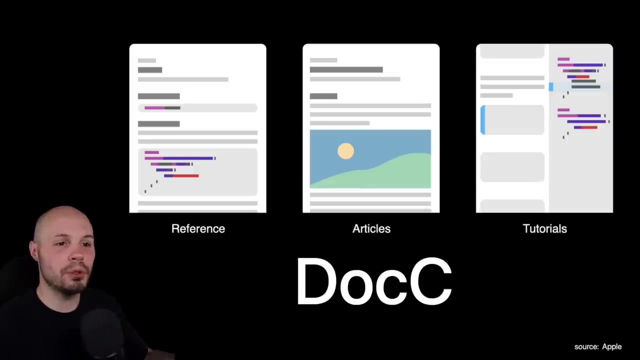 But again, it's a very, very large addition geared towards that. Okay, And then, finally, we have the documentation compiler, or doc C for short. to put it simply, this is a way for you to nicely document your code, whether it's your app or a framework. 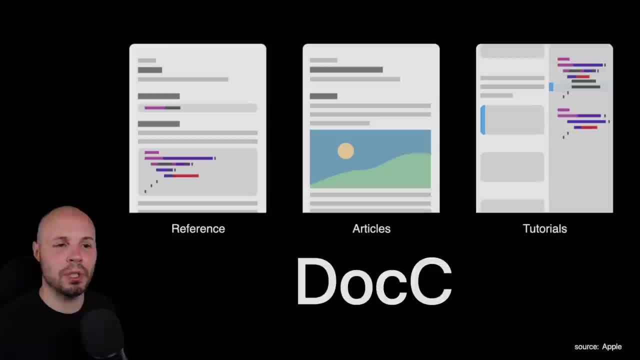 you're building that other developers are going to use to interact, just like Apple's code does, for example. you know, here I am in my cloud kit manager, right, If I was like, Hey, what's a, what's a CK query? 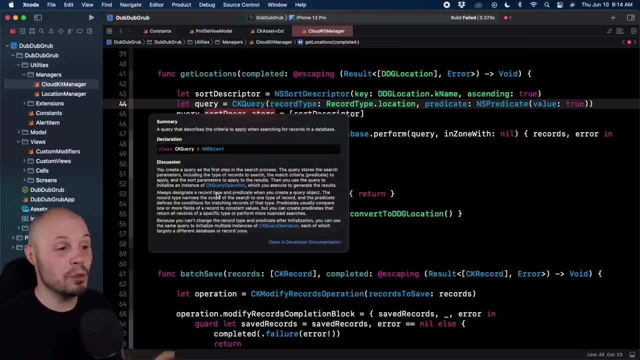 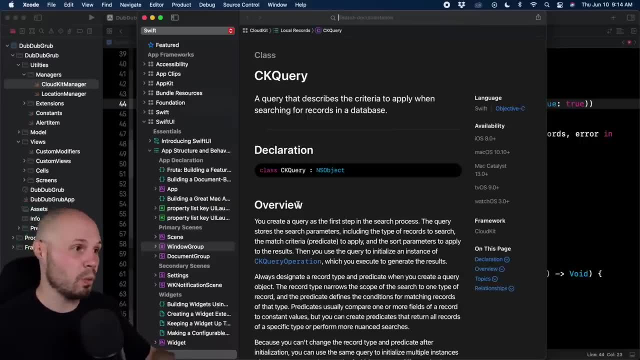 And I option, click on it and I get this little quick look. doc C allows you to do this for your own code. And again you can hit open and documentation. and there you go. documentation would show up here as well. It also allows for articles and interactive tutorials. 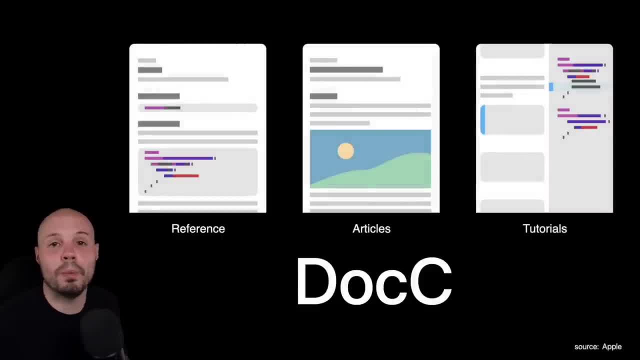 similar to Apple's own SwiftUI tutorials to be built for your code base as well. So again, I'll link to the WWDC talks in the description. but this is another big addition because we've all been there right, We've all tried to use a third-party framework. Documentation is not that great, so 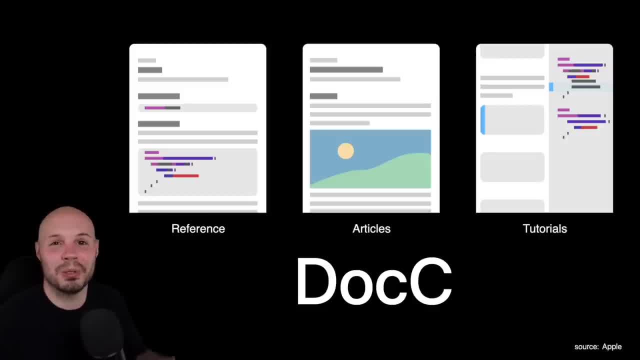 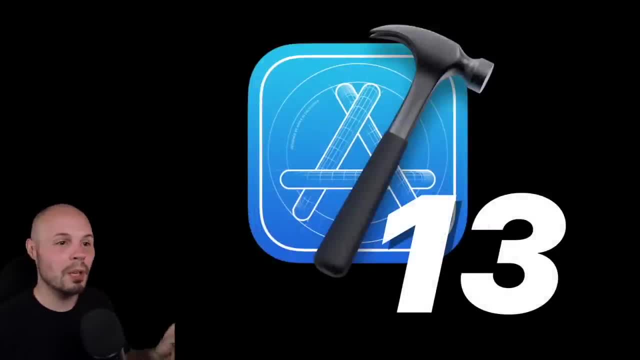 hopefully a lot of people adopt this and we can get rid of those struggles trying to deal with a third-party framework. So those are the highlights of what's new in Xcode 13.. Of course, there's much, much more. Hope you enjoyed the video and we'll see you in the next one. 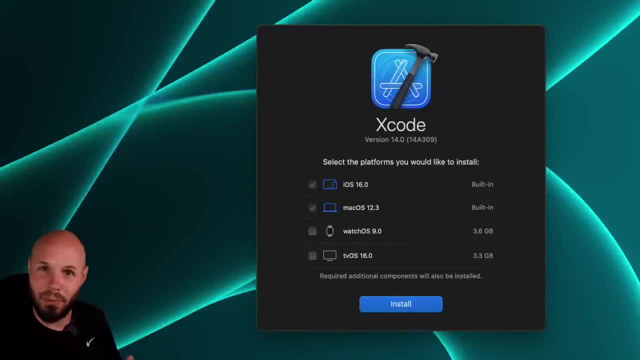 The very first thing you'll notice about Xcode 14 is that it went on a bit of a diet. By default, it doesn't include the watchOS and tvOS stuff. You just get iOS and macOS SDK. Now, of course, you can check the boxes and install those, but if we're being truthful here, just between me and you, 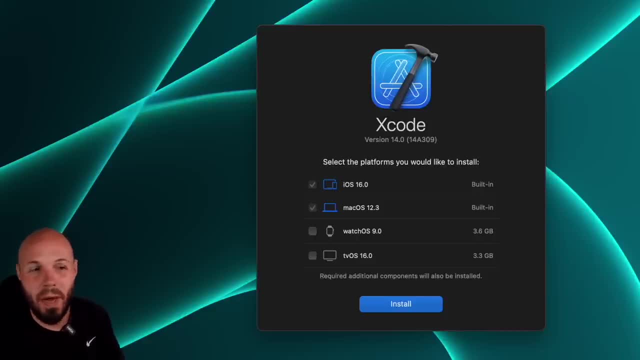 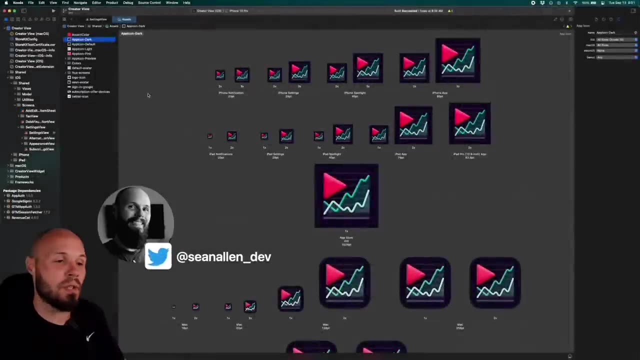 most developers aren't working with the watch or tvOS, so why include that in everyone's Xcode? So that's how we got that 30% savings and a much lighter download. The first new feature of Xcode 14 I want to show you is a very nice quality of life improvement, As 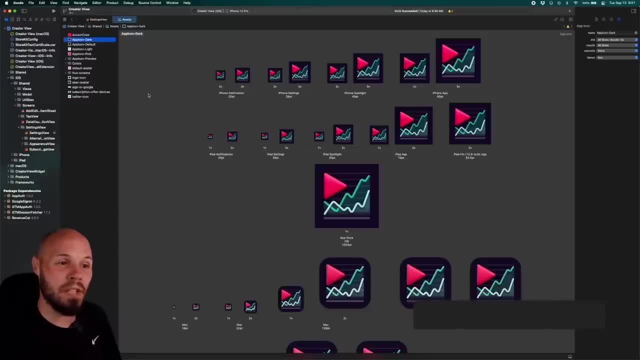 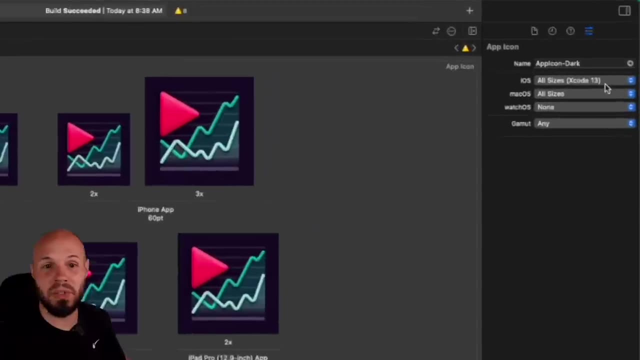 you can see on my screen I have a crap ton of icons. Now what we can do instead of having to create all these different sizes in like a design tool and bring them in Over here. on the right you can see you have iOS all sizes. Still says Xcode 13, because I guess there's maybe a slightly. different version for Xcode 14, but if you go to single size, you'll notice as long as you have the 1024 point icon, Xcode will automatically scale it down to all those other ones that you've got. So instead of having all those icons now you just need this 1024.1 and you're good to go. Quick note: 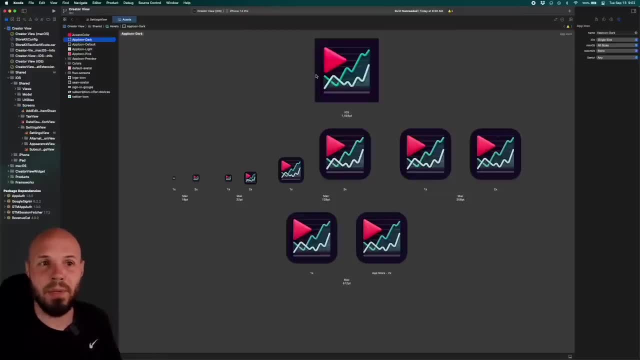 that, like I said, Xcode just scales it down, so some apps will use, you know, different versions of their icon for the super small, like 32 by 32 version, just to make it more visual. So if your app icon is like that, you might not benefit from this, but I would argue most people's app icons can just be. 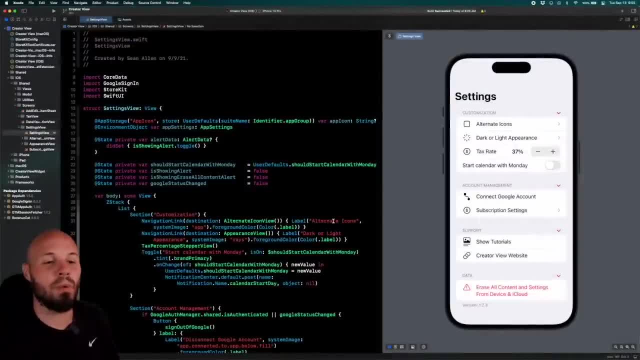 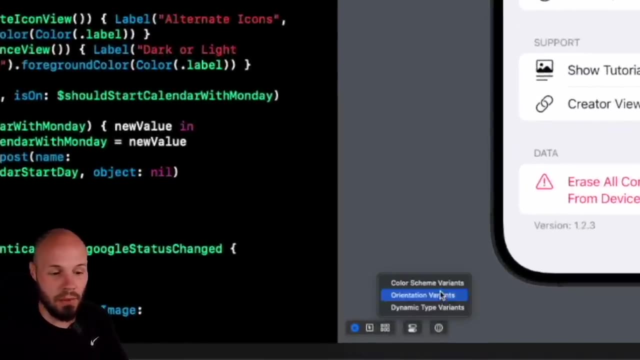 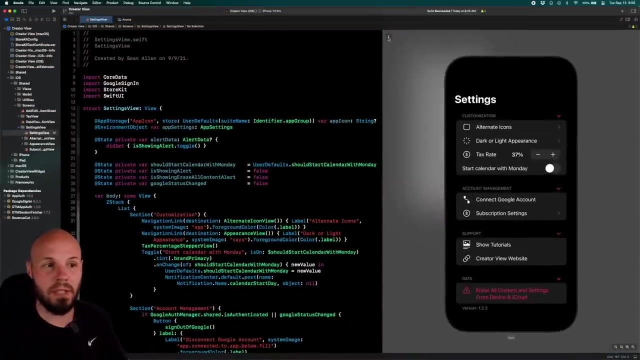 scaled down. So again, huge quality of life improvement. Moving on to SwiftUI previews: First up we have the color scheme variants And if you look at my preview right you can see you can click color scheme variants. and now look at my preview right, you get the light and dark modes side by side. 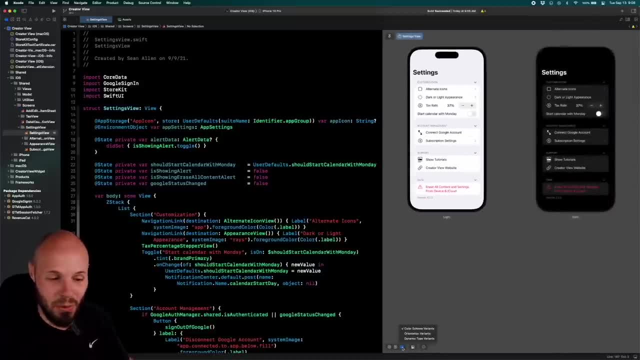 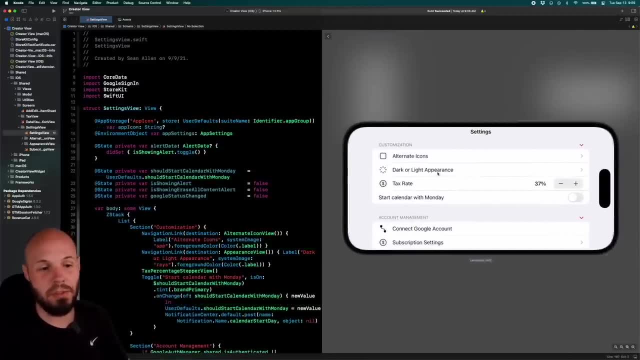 just like that, and you click on one of them to make it bigger, Then a little back button up here to go back. Click the light one if you want to really dive in. Cool, so I can see light and dark mode Orientation variants. Nice, I can see portrait landscape left. oh, if I make it bigger here Or I can zoom out of my preview, either way, Cool, I can see landscape left, landscape right, landscape left, landscape right, landscape left, landscape left, landscape left. 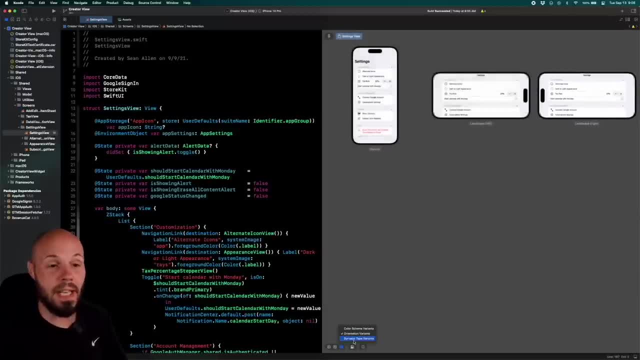 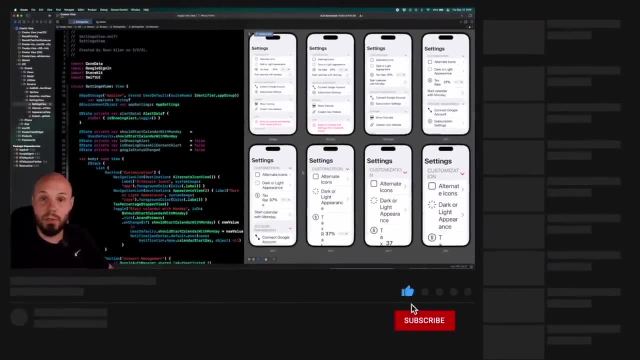 right Again, orientations, just like that. Now the really cool and dynamic type variants you're gonna see we're gonna get a bunch So you can see how your view will look with all the different dynamic type settings. just like this. Now, of course, before you could add modifiers to your previews to show the different 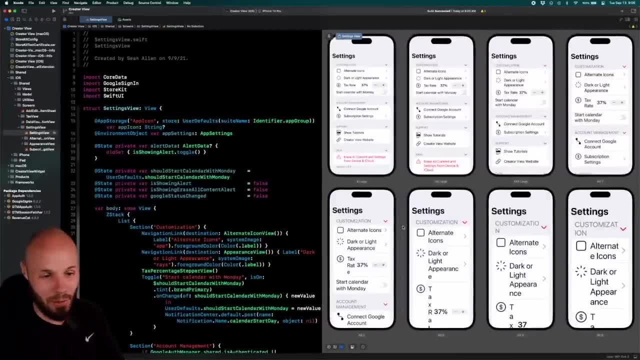 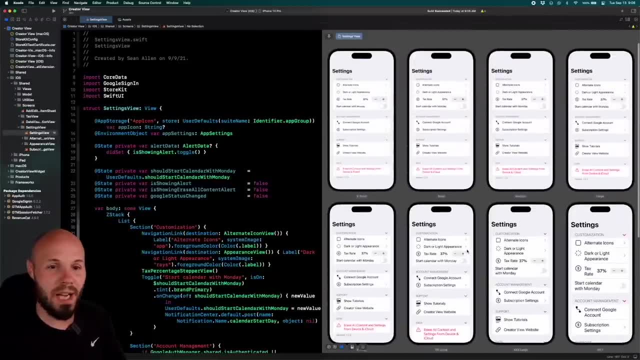 variants and have a bunch of different previews up there. This is just so much nicer: in the click of a button you can see all the variants and see what kind of work you have to do for these super duper large sizes. Now for some code. 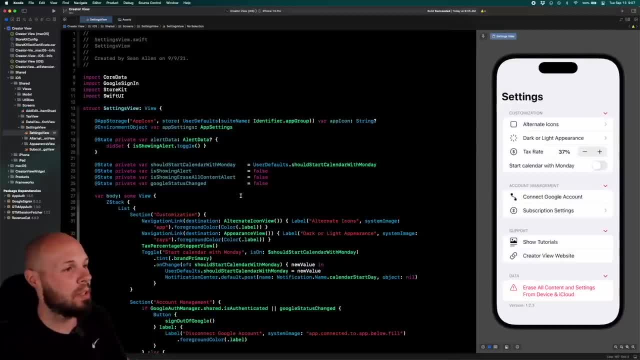 editor improvements here, so I'll make my preview smaller now, because that's not important. The first quick and easy thing I want to show you: as you can see, we're in a settings view. I'll make my code a little bigger so you can see it. 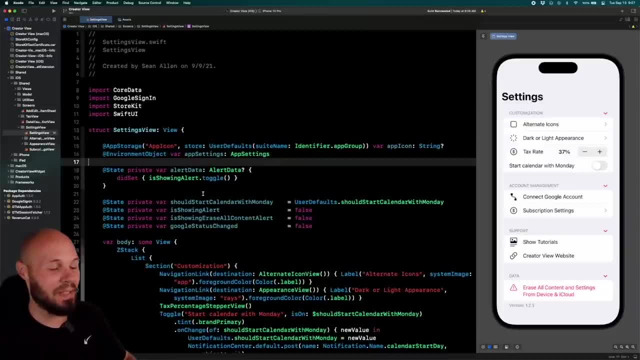 By the way, I know there's many improvements I can make to this setting screen in the code. That's not what this video is about, so keep your comments to yourself. I know there's issues. Anyway, we're in the settings view, but as you, 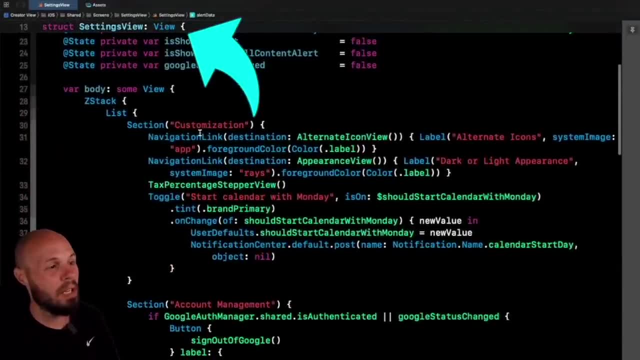 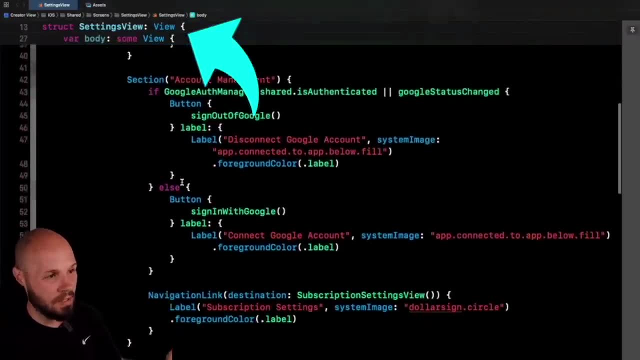 can see, we get the sticky headers. So, bam, settings view stuck to the top. and here's where it's good, because, right, my var body sum view. there's a lot of stuff going on in it. So you can see, I know that now I'm in var body sum view As I'm 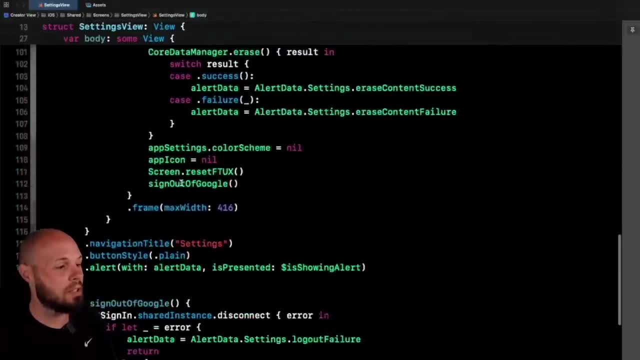 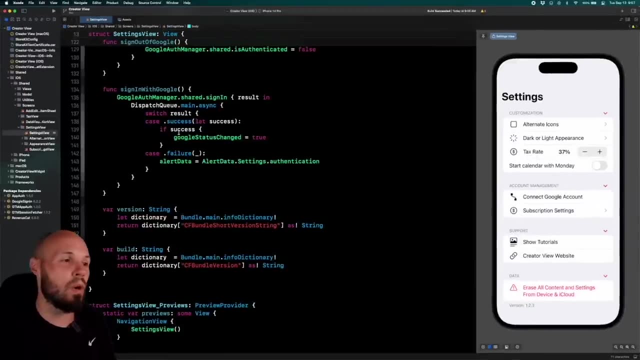 scrolling down, I'm still in var body sum view because there's a lot going on, Still going, and then now we see where the sign out of Google function here. so now that pins to the top. So that is sticky headers- A nice way to know where. 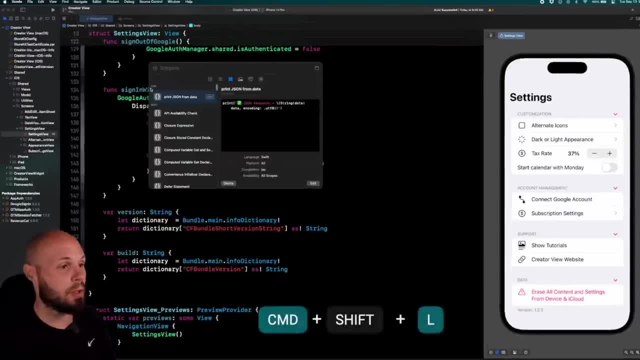 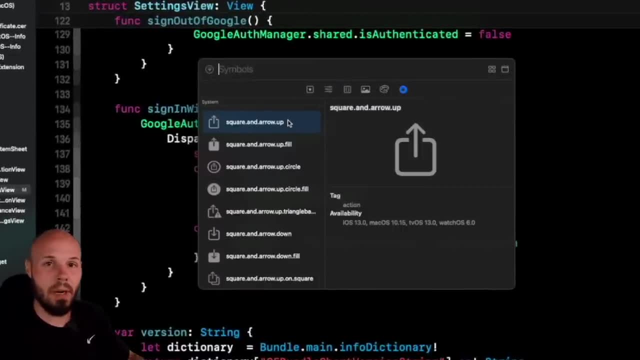 you're at in your file. Another nice thing: if you do command shift L to open up your library, and over here on the right you see SF symbols- this little star here. SF symbols are built into your library. now I don't know about you. I. 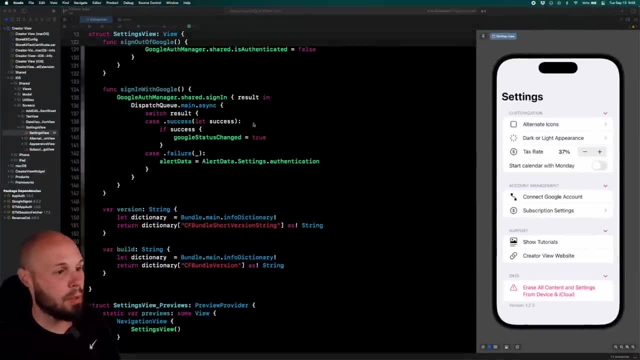 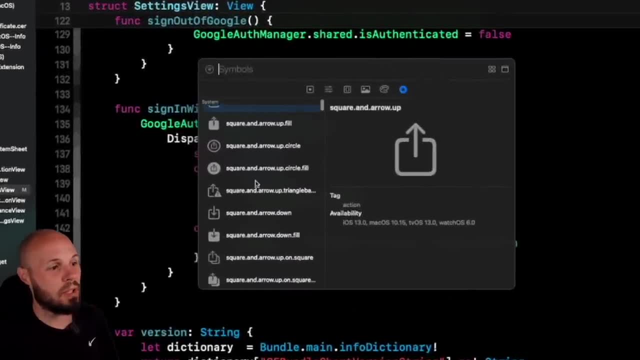 always would have to go command space. you know SF symbols. open up the app like you see here, scroll through, find them. It's just a lot of extra steps. Now again, command shift L. pull up your library, hit the little star and they're searchable too. so I can do Sun. I can see all the different Sun and 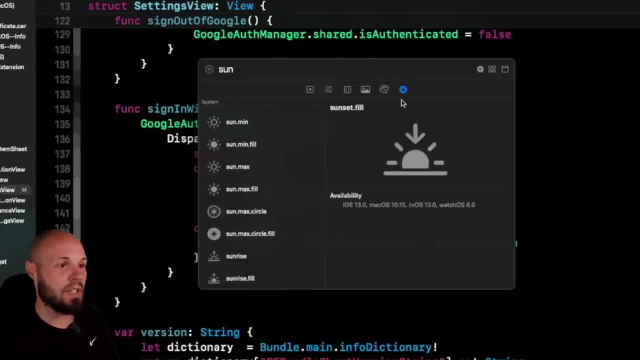 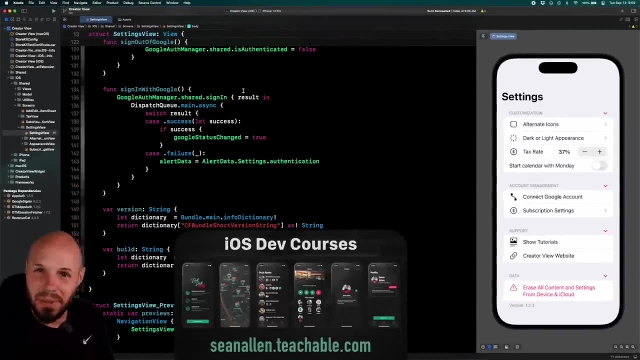 stuff like that, So nice to be built right into the library. Again, command shift L, hit the little star and you get all your SF symbols And another little thing. and I don't want to like discredit the little things, right, because all these little again quality of life. I feel like I said quality of life so much. 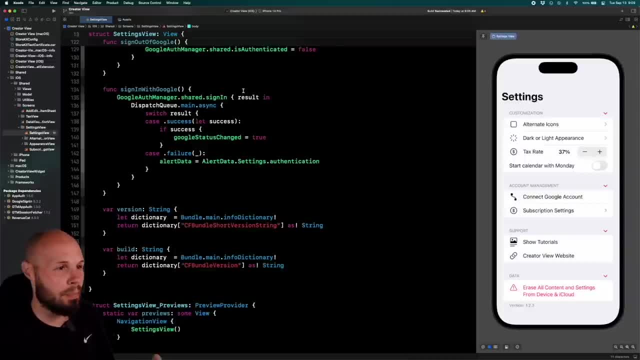 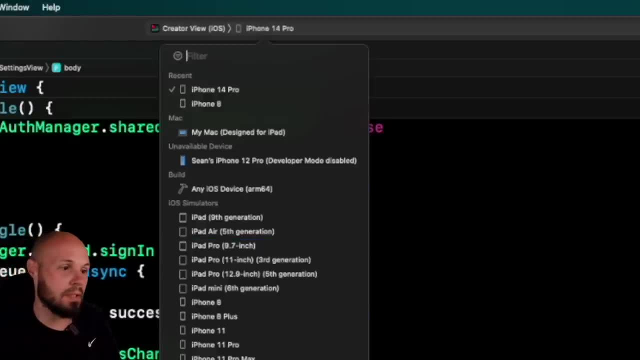 in this video. but all those little quality of life improvements like really add up to a better experience. And another one here is in our simulators. right you click on iPhone 14 Pro. you know, you've had all these simulators, you know, and if you have the watch OS and TV OS, 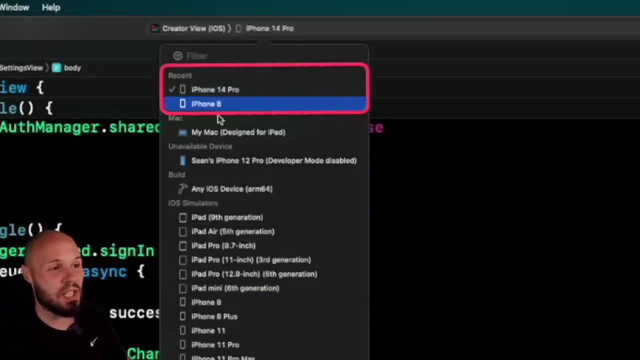 you got even more. So this is nice. we have this recent section up here. so if you're bouncing between- like in this case- you know, hey, I was testing the iPhone 8 and then iPhone 14 Pro- your recent simulator is gonna be right up there, which is again a nice improvement, And we can now see test flight feedback. 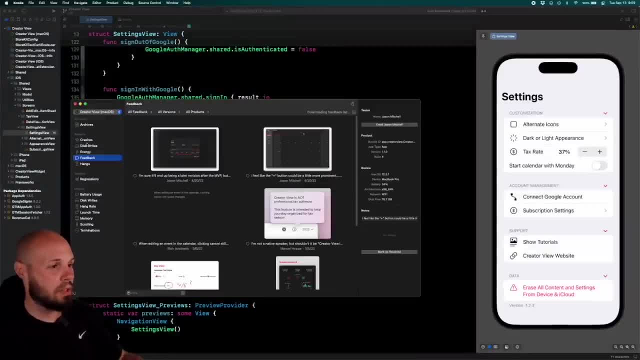 right in Xcode. So I go to Windows organizer. now this is over here. well, feedback already have it highlighted. Spoilers. you know we used to be able to see crashes, all this stuff. now I can go to feedback and I can see. I'll make this. 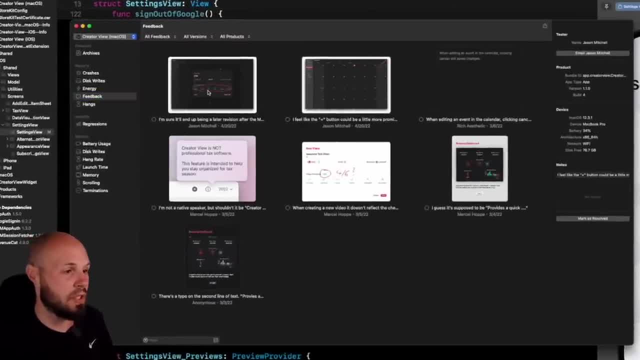 bigger here, all my test flight feedback right in here in Xcode. and you see, if I want something over here on the right I can email Jason Mitchell. But yeah, you can see all your test flight feedback right from here with screenshots, email the user. Normally you'd have to go to App Store, connect and in test flight and 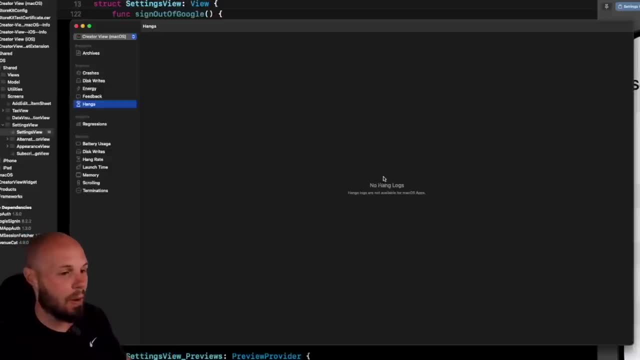 dig for that. now it's all right. here You also have the hangs. that is new. Now I don't have any hangs here. well, hangs, the hang logs, are not available for Mac OS, so I'm on. I'm on the Mac OS version. If I go to Creator View iOS, I don't think. 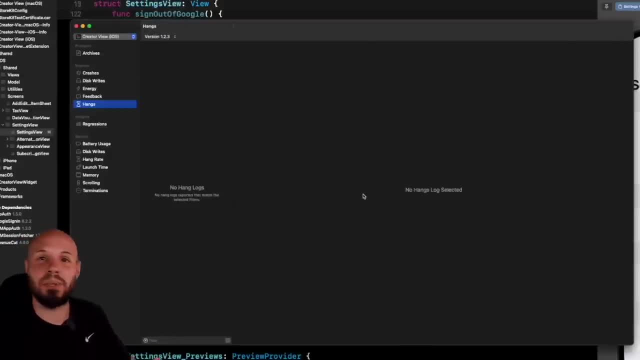 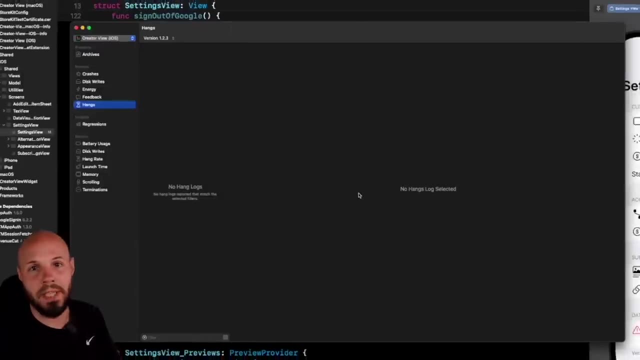 there's any hang log detected. I'm sure Creator View does have hangs, but here's a screenshot from the WWDC video of what it would look like with hangs that you can diagnose. Again. this is all new in the organizer right here in Xcode. Okay, 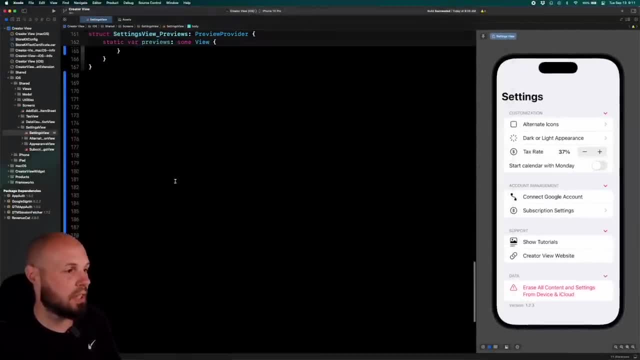 we'll close that and back to the code here. We're going to talk about some autocomplete stuff here, so I made some room, as you can see. So now we get a lot of boilerplate code done for us, like member wise initializers or codable. 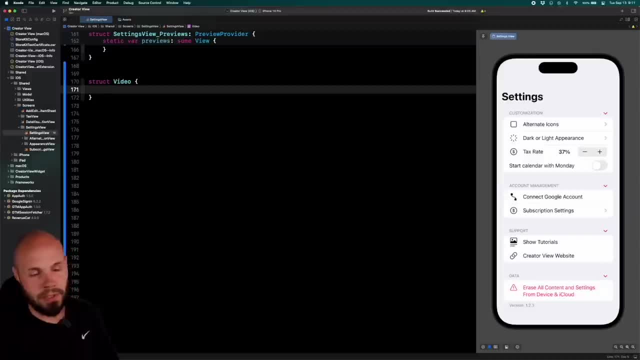 conformance. So let's say we have a, you know, video object. this is just a real quick dummy. object: bar: title, which is a string. bar date, which is a type date. bar is live stream, which is a boolean bar, note string. Now, with these basic structs, typically you have to member wise. 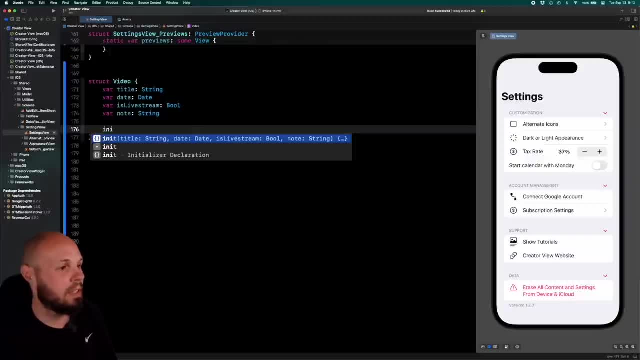 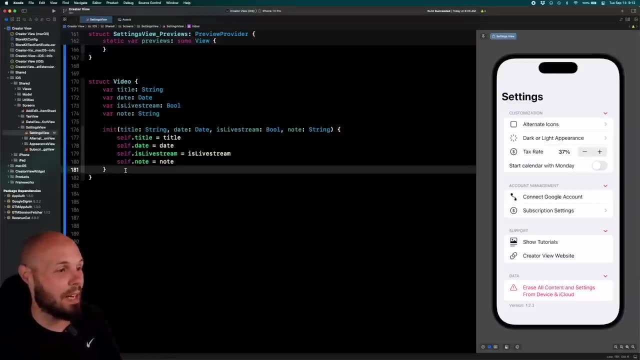 initialize for free, but sometimes you need to type it out. So you would do init and then you know. anyone that's been developing iOS for a while has typed this out thousands of times manually. Now we get that for free. Same thing with like codable conformance. So we'll conform video to codable and then you just start. 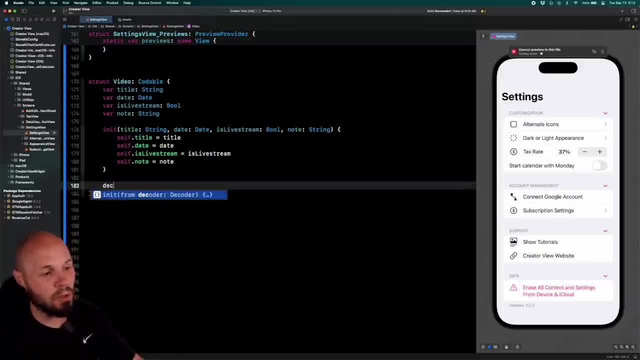 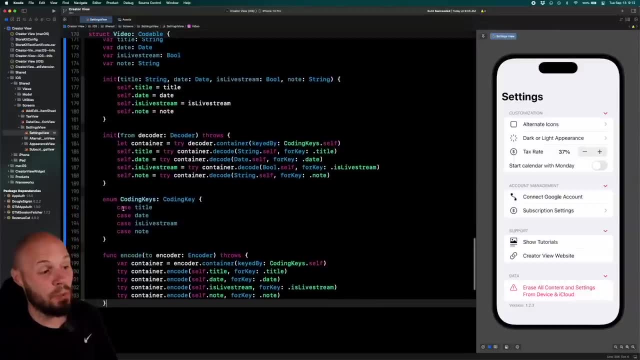 typing decoder right here, and you see, you get the little curly braces with the dot dot dot. Now you get all this stuff in there, and then same thing with type encoder Bam, and then now you also, when you do both of them, you get the coding keys. So, like I said, there's just a lot of boilerplate stuff. that again, if 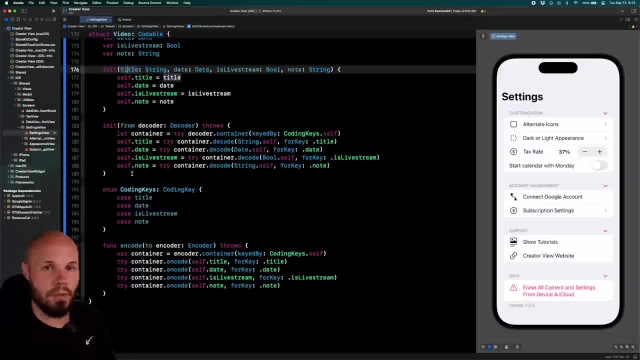 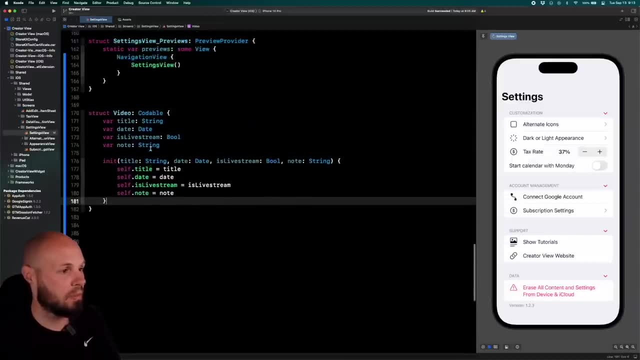 you've been coding for a while. you've typed this out manually plenty of time. The last thing I want to talk about in this section is the auto completion of parameters. Let me get rid of all this codable stuff, just to declutter the screen and not be so confusing. So you know, a title for video is cool, a date- 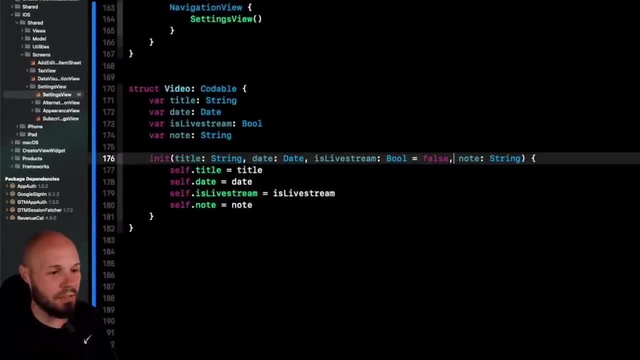 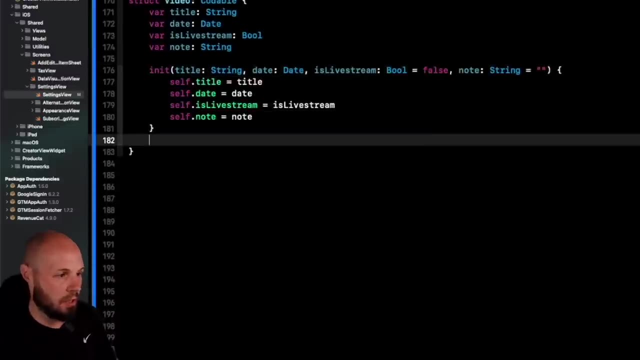 for video, a live stream. Most it's not gonna be a live stream, so we can set a default value to false and then a note. Most of them are gonna have notes, so I'll have a default value of string. So now let's say we had a function here. 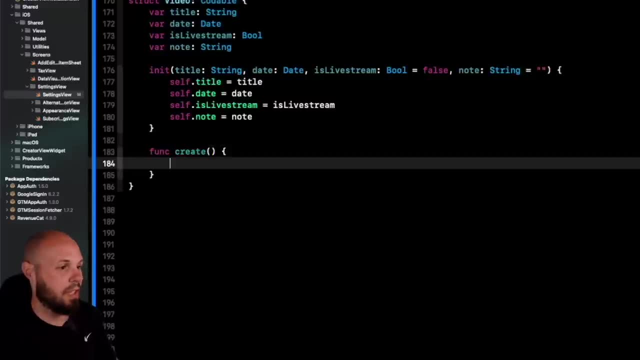 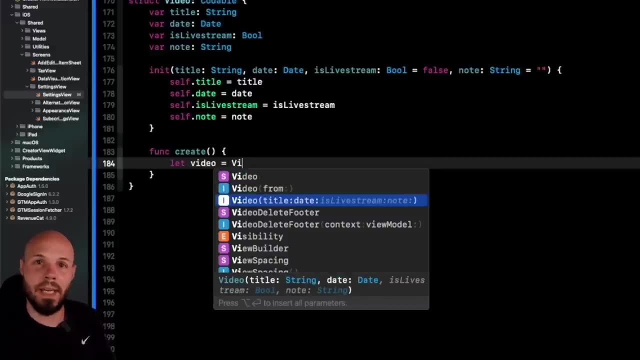 again dummy, dummy code here: func create and in here we're gonna create a video. So let video equal, then we'll initialize a video here. Now you can see down here in this: one is live stream and note is kind of grayed out and italicized. So if I just hit return, because those have, 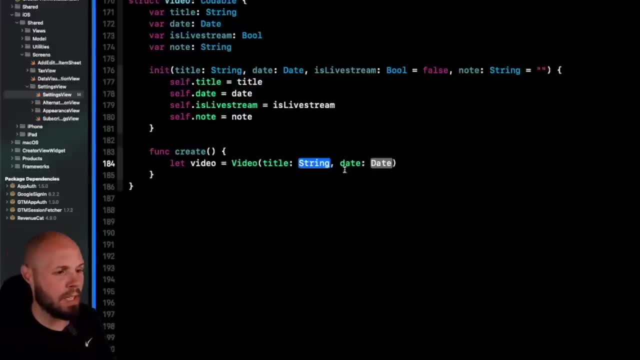 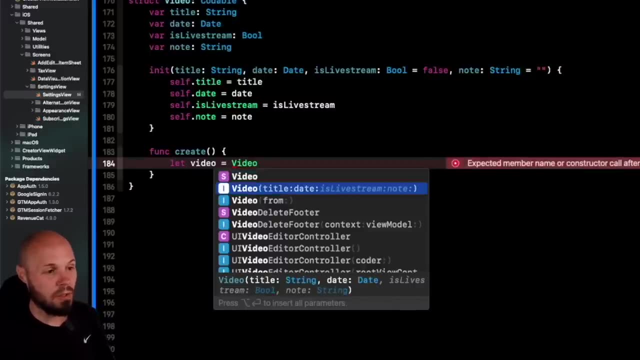 default values. bam, I just get title and date. But if I go back here, what if I did want those values? There's a couple ways to do this. So video and then, if I hold option, you'll see they light up and I'll get them all. So if I hold option, hit it. 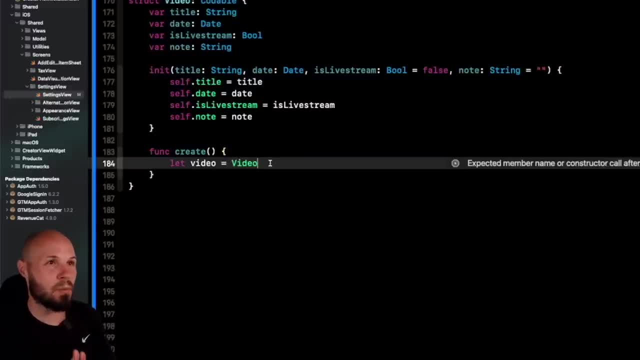 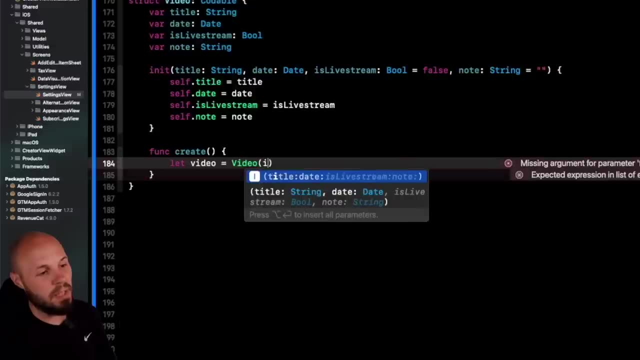 get them all Cool. Now. another way to do this real quick- and this is really gonna come in handy in SwiftUI, which I'll show you in a second. but if you do, cool is live stream and note are optional, But if I start typing is live. 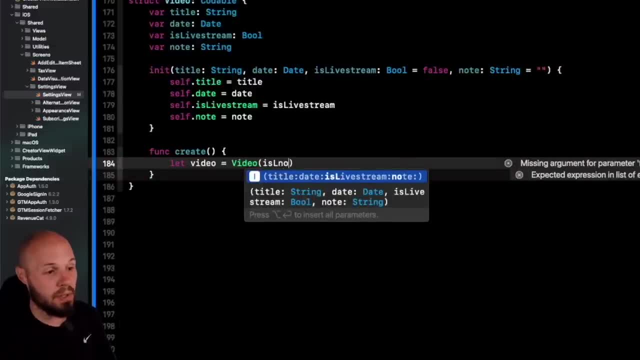 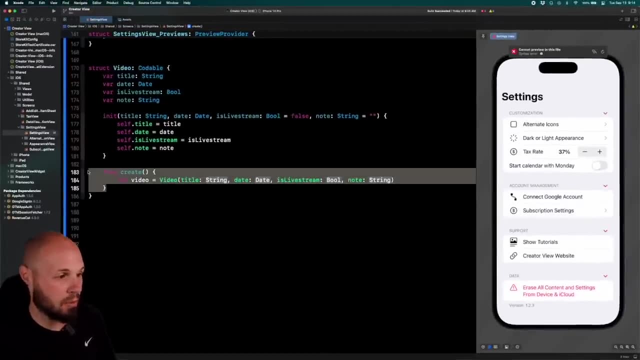 stream. you see, that will light up, and if I start typing note, that will light up as well. So now I'll get them all. Now that may seem like a contrived example when you're initializing those, but let me get rid of all this and go back to 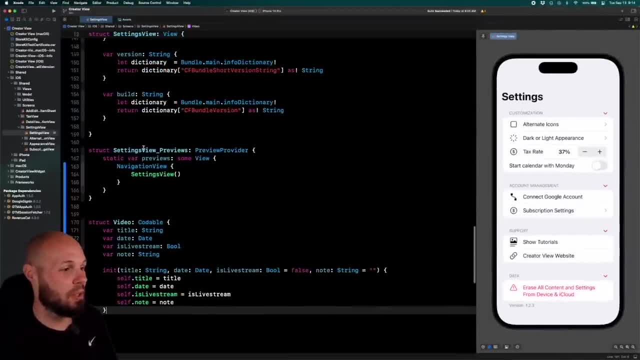 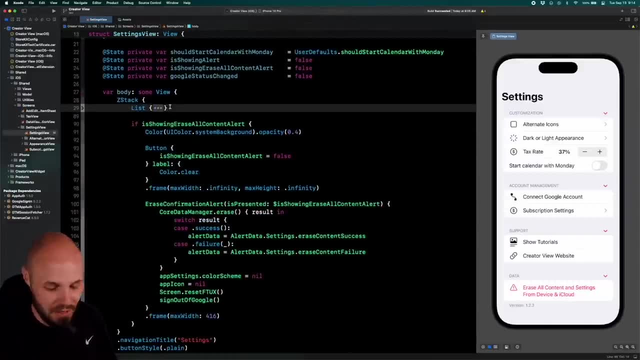 SwiftUI, and this is where this is gonna be such a lifesaver. So back up here onto this list. here for the settings view, I'm gonna code fold it so you don't get distracted by all the messiness going on in there. So look on. 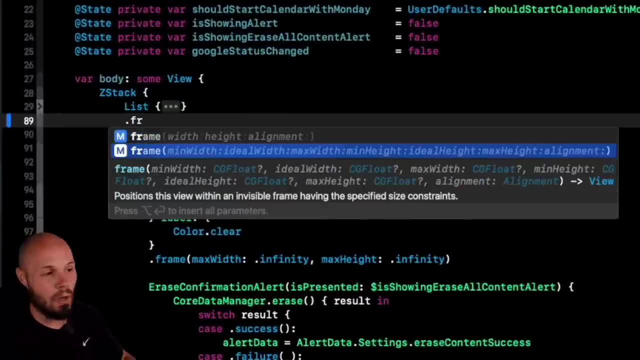 this list right? a common thing we do in SwiftUI is dot frame. Of course, if you're doing dealing with like min width, max width, there's a whole bunch of them, but this is where it's nice, where you can type it like I said. So if I did, 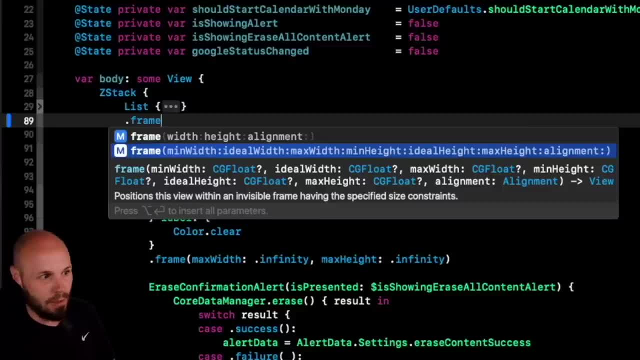 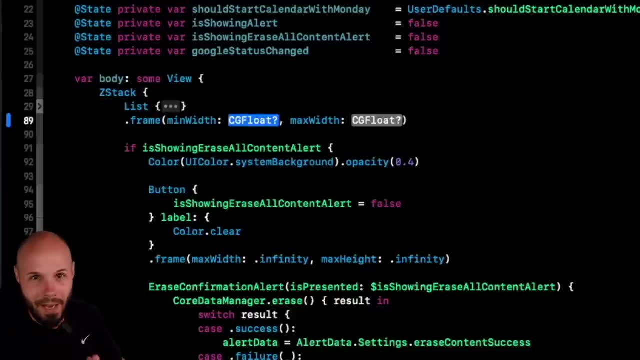 frame. again, you can hold option to get all of them. most likely you're not gonna want all of them, but if you just start typing, you know min, max. you see min width and max width lit up. I can hit return min width, max width. I know if. 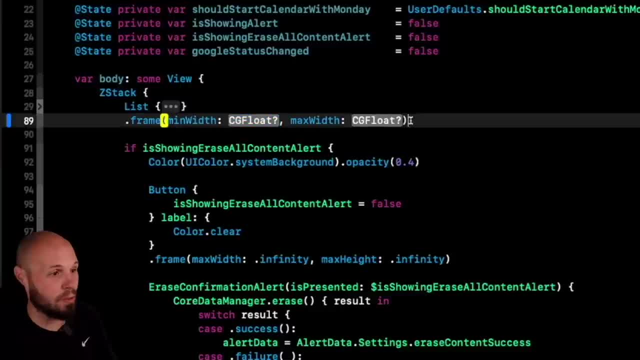 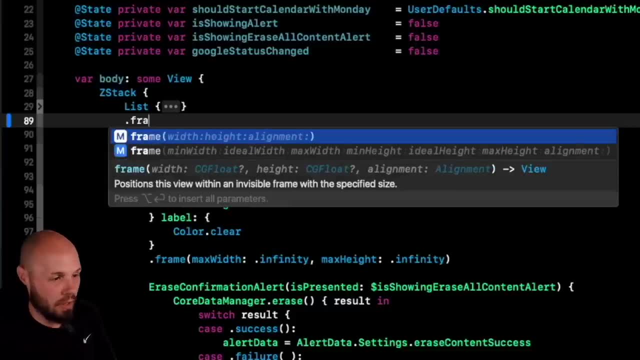 you've been dealing with SwiftUI for a while, you've had to type that out manually because you didn't want all those parameters. so that is nice. and then an even quicker one, right? so, dot, say, I just want to have the width of a frame, so, dot, frame, I don't want width and height, so just start typing width, bam. 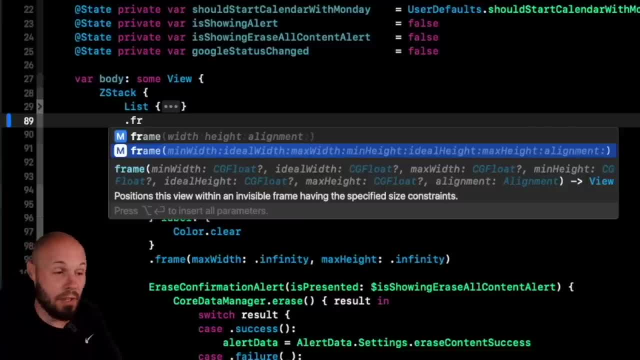 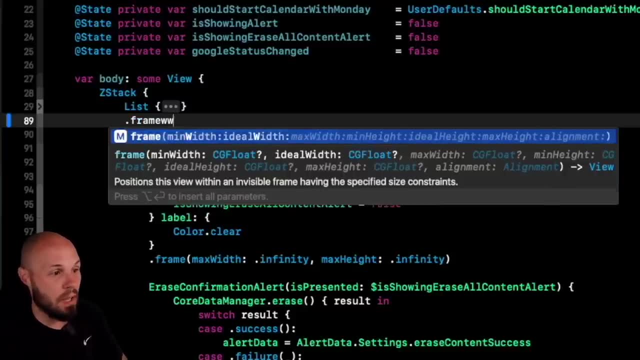 so, like I said, SwiftUI modifiers with a ton of optional parameters. you know this is very common in SwiftUI, this typing out which parameters you want. you don't type it all out, you just have to type a letter of it. so you see, I just typed a W and then maybe another W, so now I'm getting how it's going through. 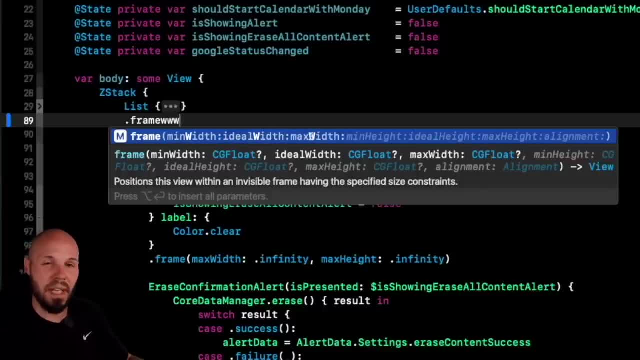 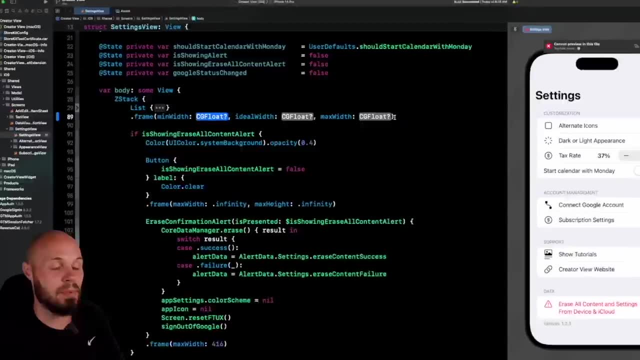 the third W. so I got min width, ideal width, max width. so there's different letter combinations you can type to get what you want. you'll have to experiment with that, trial and error with that, but that is gonna be such a time saver for SwiftUI. 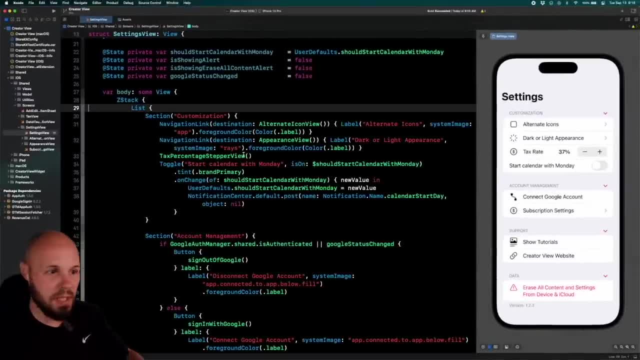 and then the last thing I want to show you is the build timeline so you can diagnose. you know, why is my build taking so long? you can really check it out in a visual manner. so before I do that, I'm gonna do a command shift K, maybe just be command K, I don't know. whatever, clean my build. 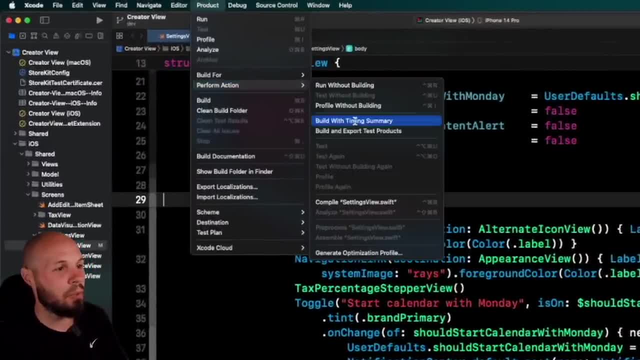 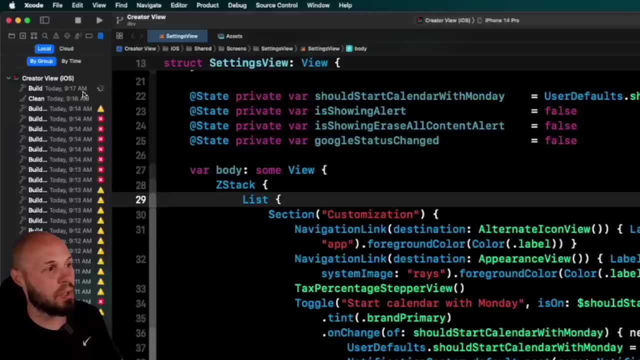 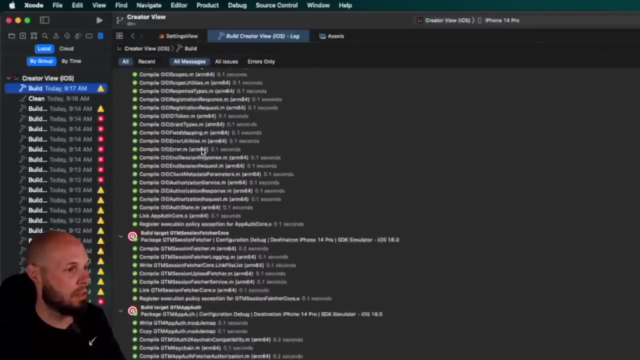 folder: product: perform action build with timing summary. so you click that, it'll build. over here on the right we'll click this to see our latest build. so you see 917 build is currently working. once that is done, building, I will show you the timeline summary. okay, so the build at 917 am is done. we click on it. I'm. 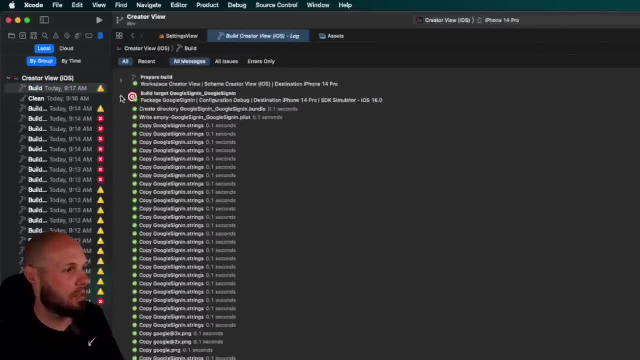 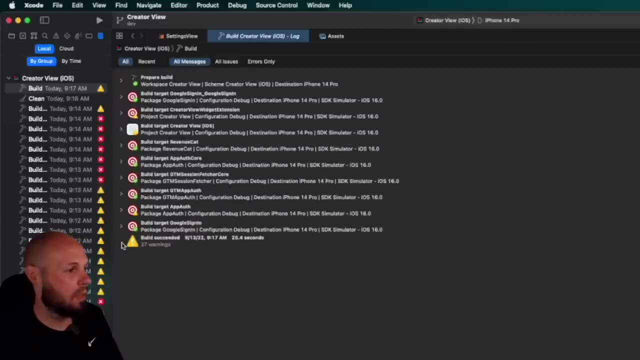 gonna collapse all this stuff real quick, just so you can get the summary here. so there's like the build right, building all the targets, building all the the packages and stuff like that, minimizing these so you can help or see it okay. so that's like the overall summary. now I don't see my build timeline right now. it 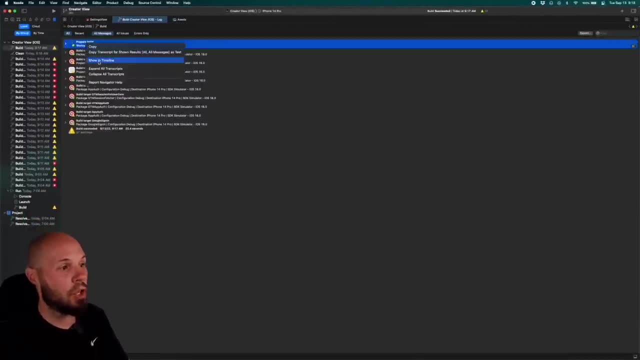 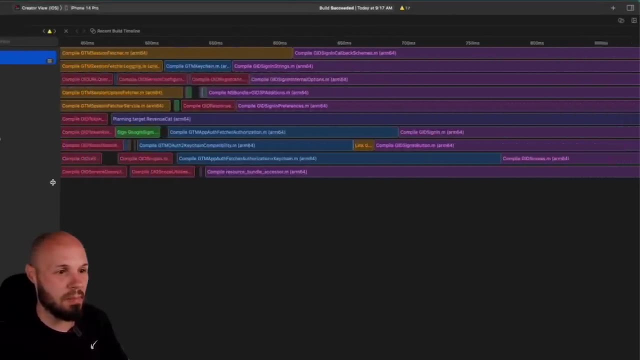 may show up by default for you, but if you right-click show in timeline, okay, put this on the right. depending on your monitor setup. maybe you want to blow, maybe you want it on the right. I guess this is big enough I can have it on the right. when I was testing this on my laptop, I just had it had to put it below. 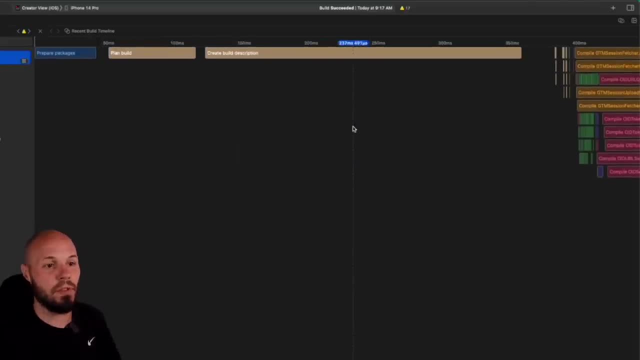 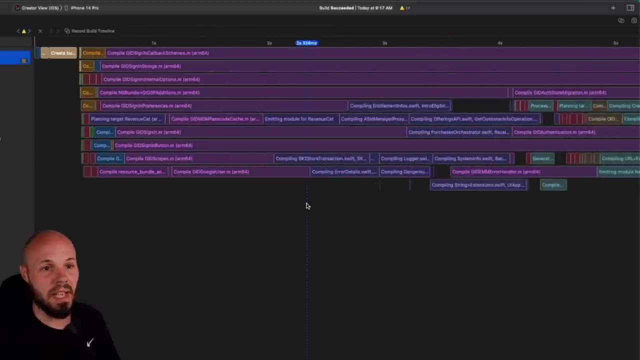 but you can see the timeline and it is in milliseconds. right now, if you hold option and kind of scroll in your mouse wheel, you can kind of zoom in and zoom in. so I'm doing it here. so instead of milliseconds here, let's do you know by. 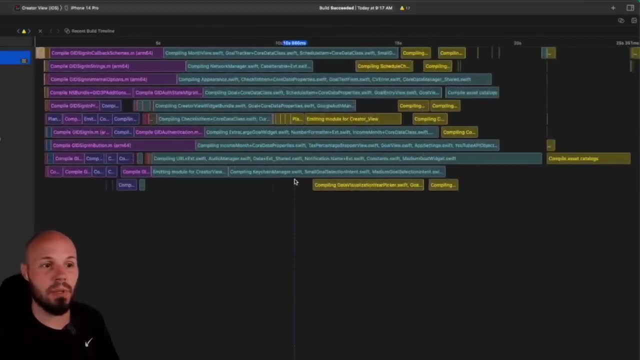 the second right, or you can keep zooming in, maybe every five seconds, right, that'll really put up the summary of your build, but you can look and see, like, what is taking so long to build, or you know, if something is egregious, something is really uh, out of whack, like sometimes your, your asset catalog can be like: 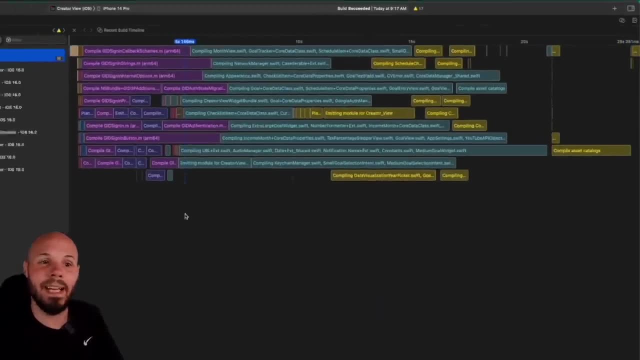 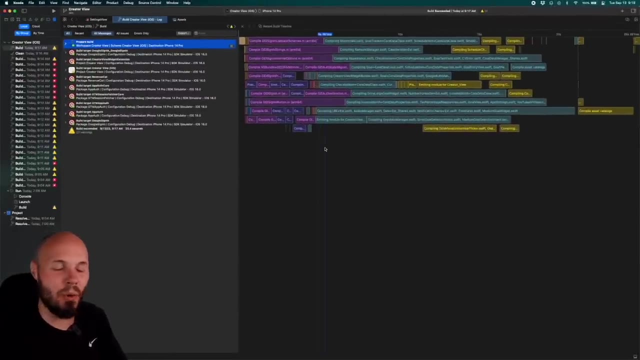 super duper long, but anyway you can see the build of your timeline to again diagnose any issues you have and optimize your build times. those are the highlights of Xcode 14 that I thought you would use, you know, on a day-to-day basis. of course there are tons more. 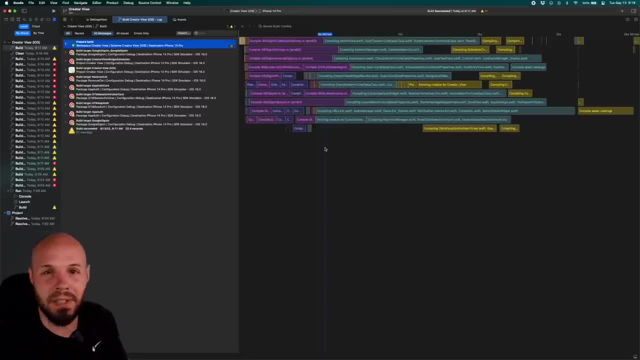 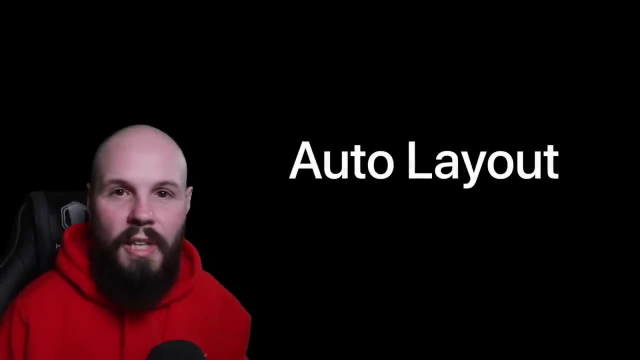 changes. I'll link to the release notes in the description. check those out if you want. we'll see you in the next video. before we start playing with storyboards and building our own apps, let's talk about what auto layout is. as you're familiar with, there's tons of different. 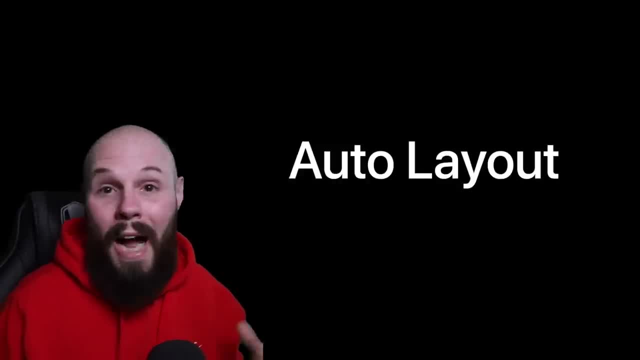 screen sizes: right, the iPhone SE, the iPhone 11 Pro, iPads, various different iPads. right, there's a lot of screen sizes developers have to handle, and that's what auto layout does. it's a constraint-based system that really makes our lives easier when adapting to all these screen sizes. and without auto, 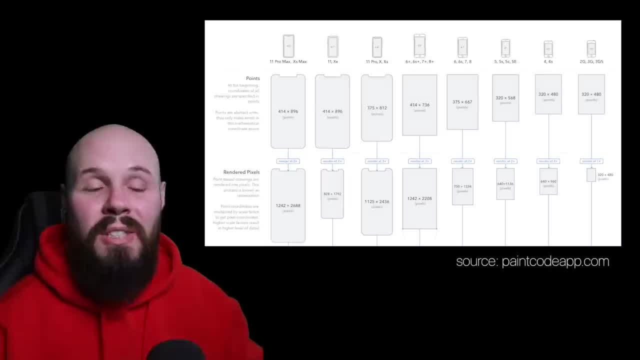 layout. we would have to create unique layouts for each different screen size, like: look at this diagram of all the different screen sizes. we would have to be like: hey, on the iPhone SE or five screen size, this button should be, you know, 10 points from the bottom. but on the iPhone 8, which has a much bigger. 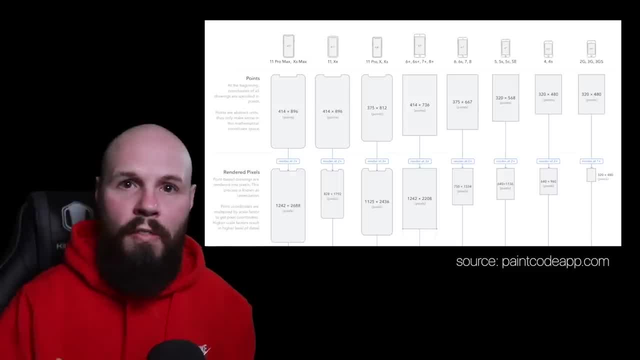 screen it should be 30 points from the bottom, but on the iPhone 11 Pro, which is even bigger screen, it should be 80 points from the bottom, and that's only one vertical layout of one element like that, so that way we can imagine your whole UI being different per screen. so 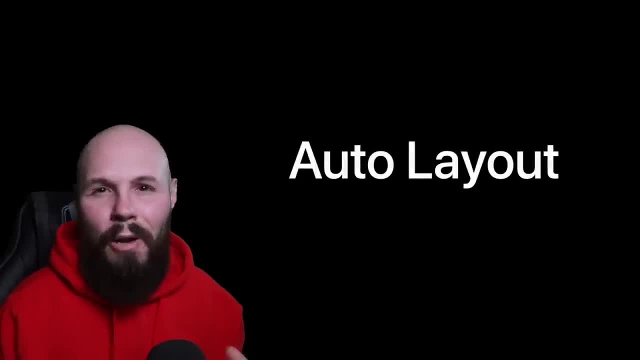 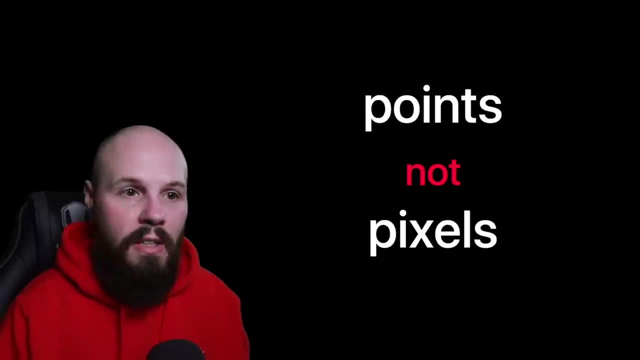 it looks good on each screen. well, thankfully we don't have to do that and, again, auto layout is the system that allows that. now you may notice when I was describing that, I said points and not pixels, and that's because the various different screens in the iPhone iPad family have different resolutions. 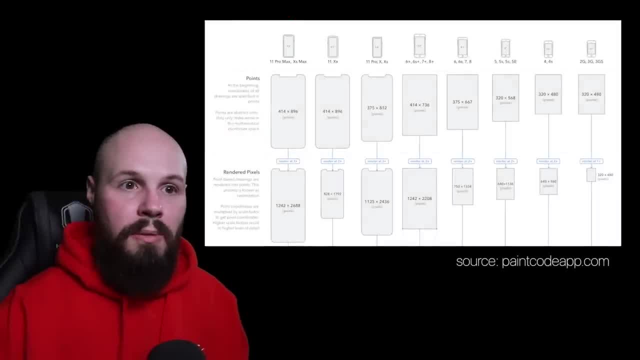 so, again, to make our developer lives easier, instead of trying to remember like, okay, this screen is a you know 3x resolution or this one's 2x, so now my screen size is a little bit bigger than this screen. so again, I think it's a good. 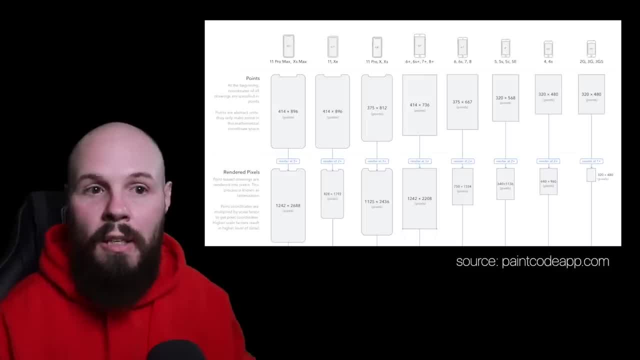 idea to just deal in points and, as you can see on this diagram that breaks down, you know the- the height in points, the width in points for each screen by just dealing in one measurement, if you will called points. that again makes our lives so much easier. we don't have to worry about different resolutions. that gets 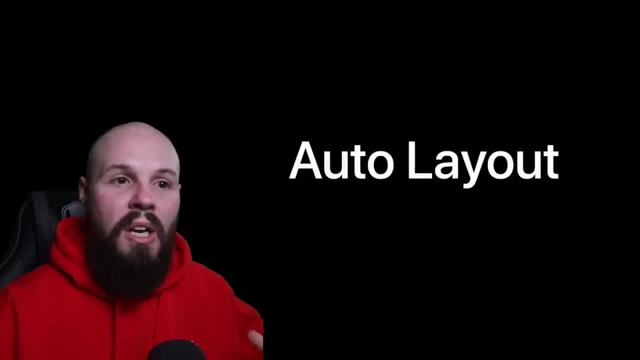 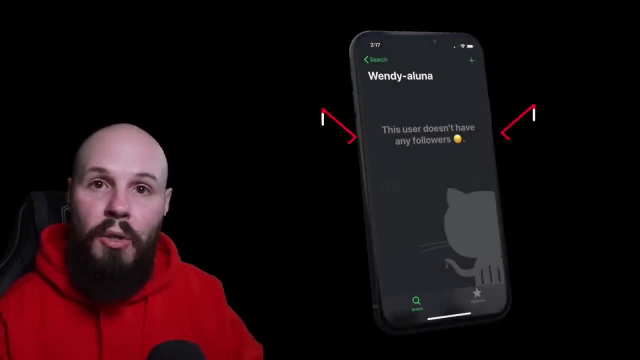 handled for us. so, like I said, auto layout is a constraints based system that helps us lay out for all the different screen sizes. what that means is, let's say, I have a label and I want to constrain it so that it stretches, so that it's going to have a 30 point padding on the left of the screen gap. 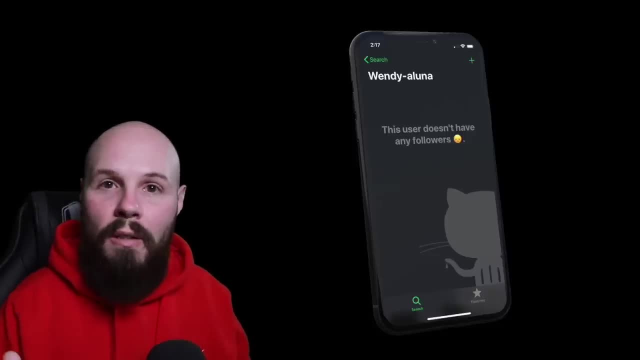 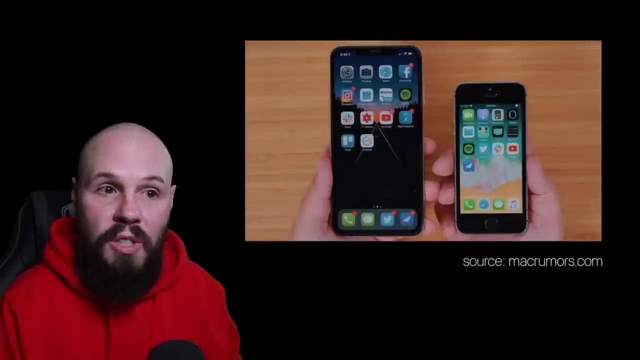 and then 30 points from the right of the screen gap. right, we want some padding on each size. well, the width of that label is going to be different based on if it's the iPhone SE, which is pretty skinny, or the iPhone 11 Pro, which is. 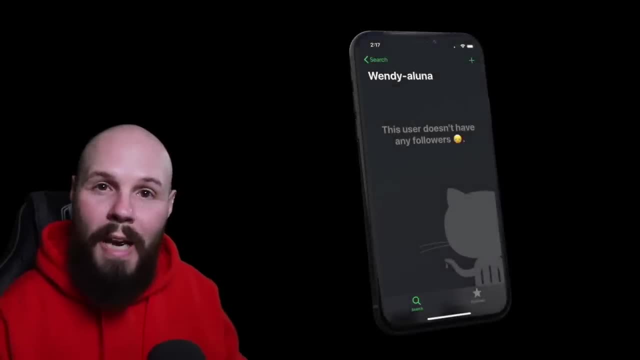 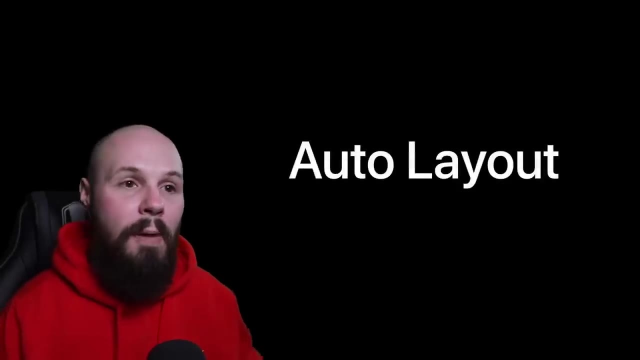 actually a pretty wide phone right. so that label will stretch, so that it's going always going to have a 30 padding on the left and a 30 point padding on the right. so that is a quick example of how auto layout adapts. or if you say hey, 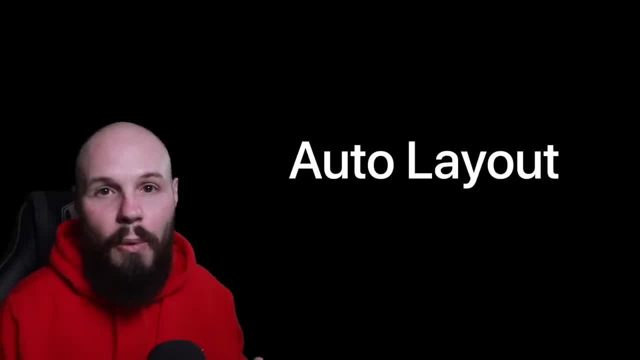 center this vertically on the screen is it's going to Center vertically. we don't have to say you know the specific point, coordinate where that should be. so that is a super basic example of auto layout. again, we're going to be using this in future videos while we build our 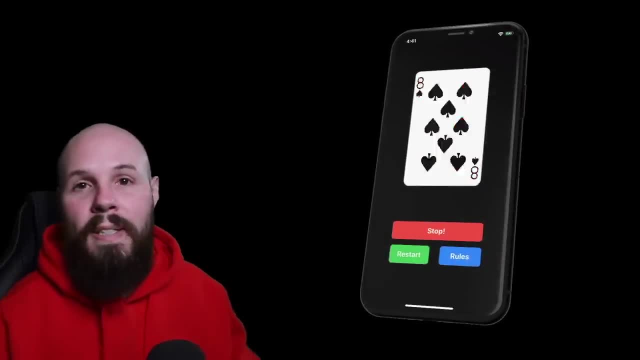 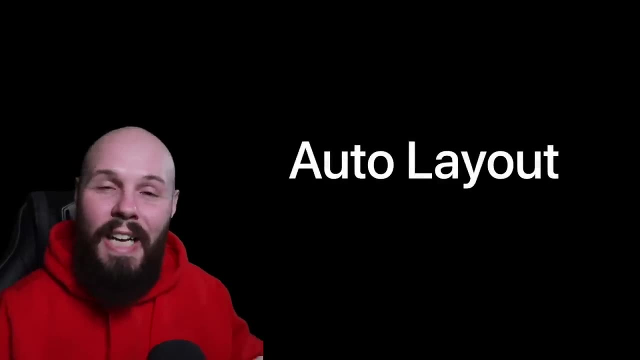 apps. so you'll get a chance to actually play with it, and I'll be explaining it more in depth as we get into it. but again, I wanted this video to just at least tell you what it was, and it's that this auto layout thing exists and kind. 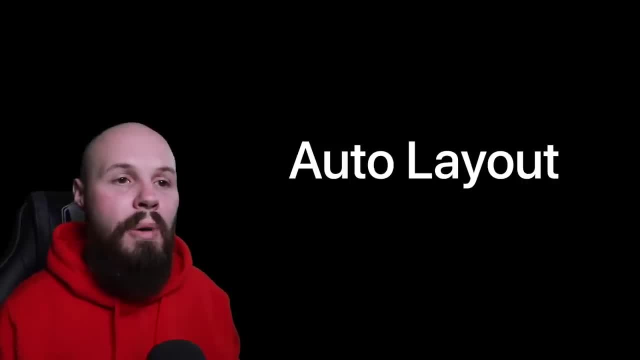 of the idea behind it. one quick thing before we move on, though, is that auto layout, while it does help configure your layout, so it gets on all screen sizes, is great. it's awesome, but it will get you 90 to 95% of the way. what that means is, if you want your layout to look really, really great, 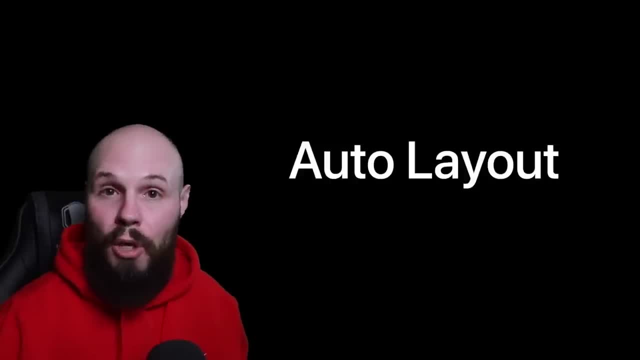 on, you know, the iPhone SE all the way up to the iPhone 11 Pro Max, which is, you know, the big phone, right? that's a huge difference in screen size. again, auto layout will get you almost all the way, but you're probably going to have to. 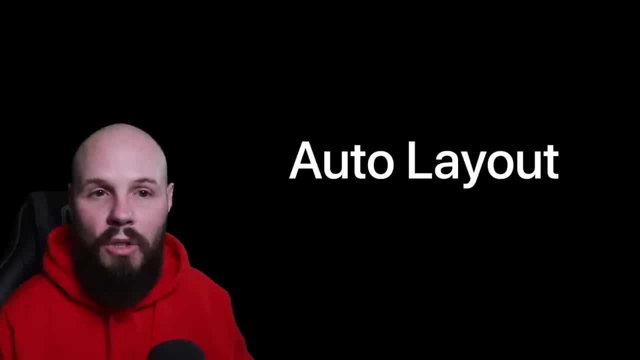 tweak manually to get your layout work looking exactly like you want it to look. and I just say that so you know in your head, auto layout doesn't do everything for you. right, it'll do almost all of the work, but you're likely going to have to dive in and manually tweak certain screen. 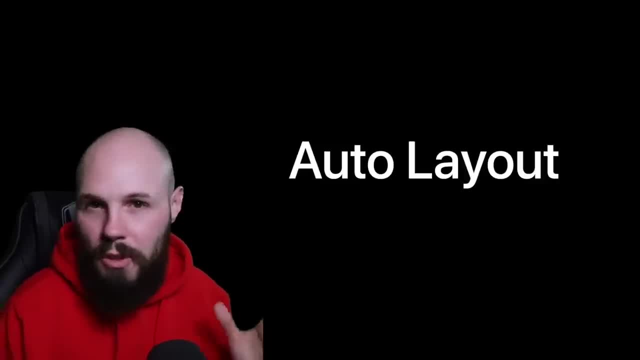 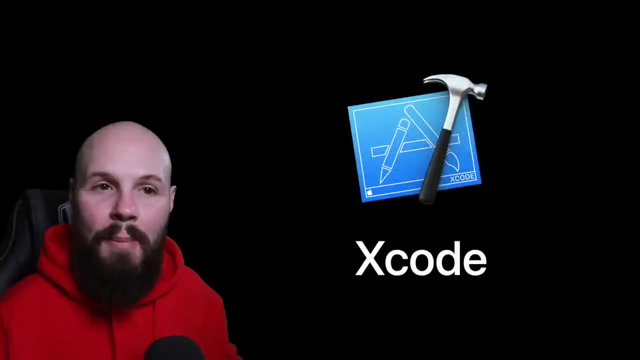 sizes to get it to look exactly how you want. so just keep that in mind. it's not the end-all be-all. it's going to do a hundred percent of the work for you. but again, it's great, all right. moving on, when building our apps in Xcode, we're actually building our apps on top of a. 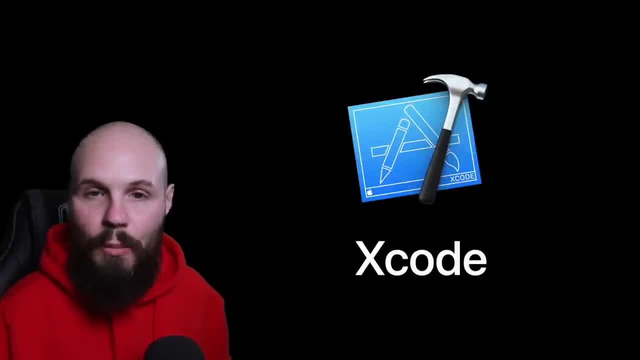 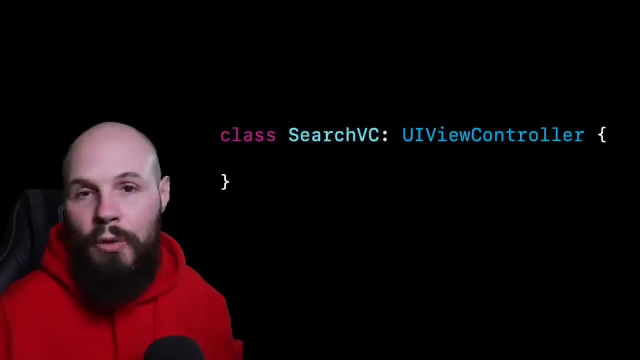 foundation that Apple has already built for us. remember, in previous videos I talked about the GF button. that was a subclass of a UI button. he even talked about, you know, subclassing a UIView controller. well, that's an example of that, like all the button functionality like is already. 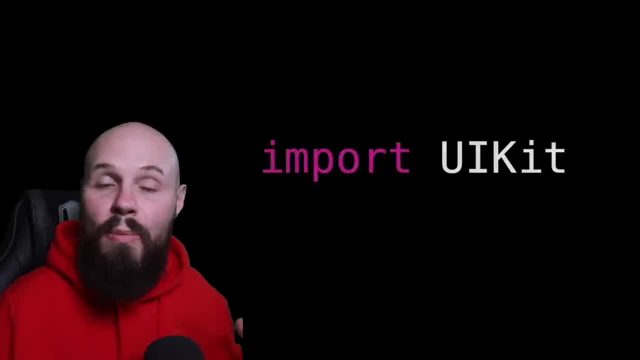 built by Apple. we're just building on top of it and that framework that we're using- it's called UIKit, you'll notice- is it was UIButton, UIView controller, like anything, with the prefix UI means it's part of UIKit and we're going to use those components to build. 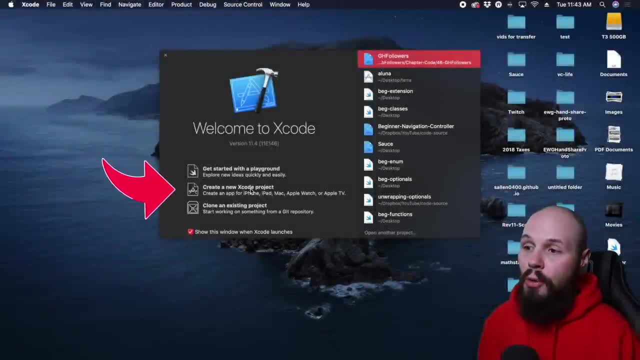 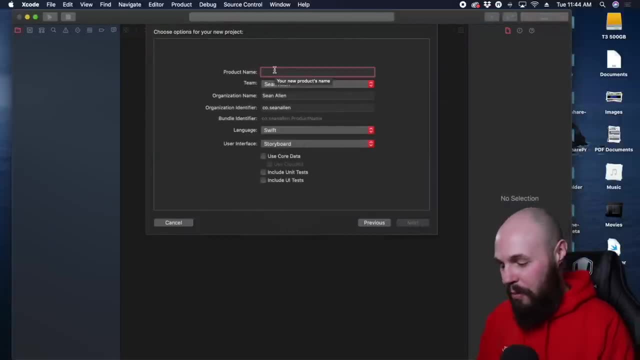 our user interfaces, so open up Xcode. to build our user interfaces, so open up Xcode. up Xcode. create a UIкт, new Xcode project and a single view app. not sure if you've deleted your previous test one that we use, but we can call this UI kit intro if you want to call it. 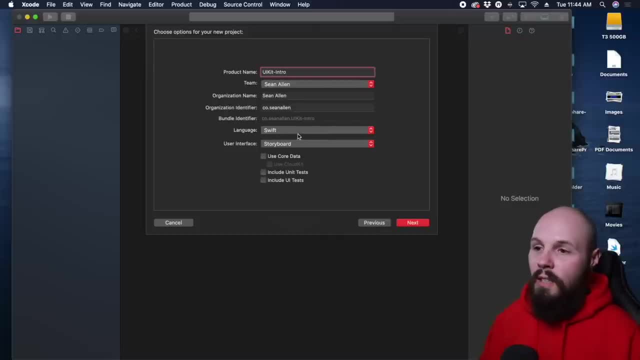 that again: team. make it your own organization name, make it your own language. Swift user interface storyboard so we could do Swift UI or on that later. right now we're gonna make sure you click storyboard and then we don't want to do objective C, we want to do Swift and we're not worried about unit tests. 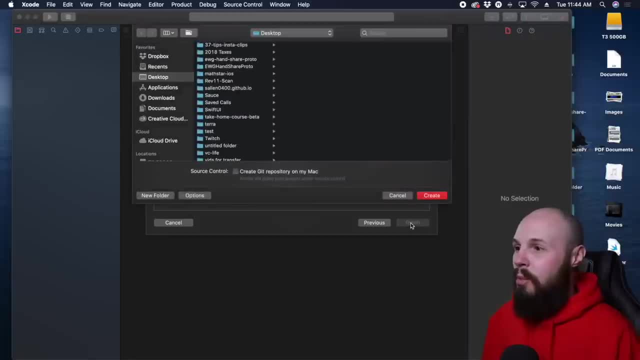 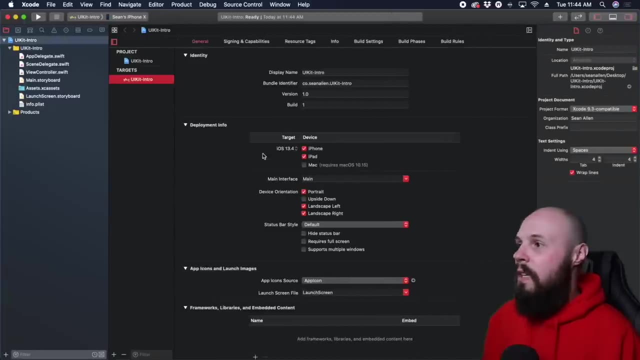 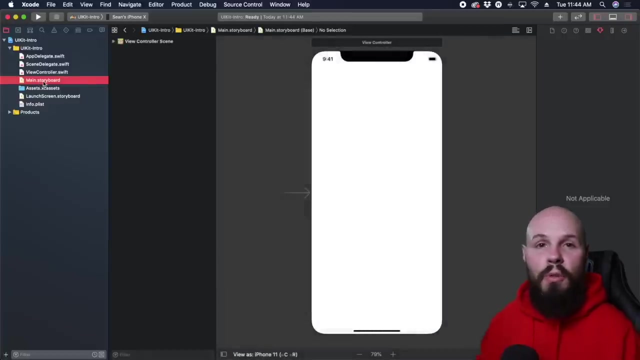 or core data or anything like that. so hit next. that will create this project. save it to wherever you'd like to save it. I'm just putting mine on my desktop and let's make this screen fill up here. so now click on main dot storyboard here on the left. here we are. here's our first view controller, this arrow right here. 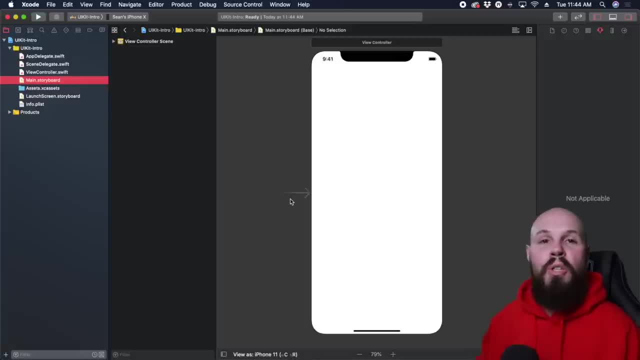 means it's the initial screen on the view controller, so this is what shows up first. now, to put it super simply, a UI view controller controls views on your screen to display. you're going to want to make sure that. you're going to make sure that you're. 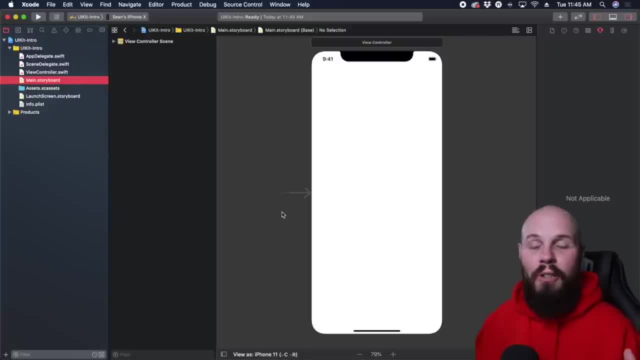 going to want to make sure that you're going to make sure that you're going to. and most of the time a view controller is an entire screen. you can create reusable child view controllers. that's more of an advanced topic. just know that that is possible. but for the sake of this course, very beginner, our view. 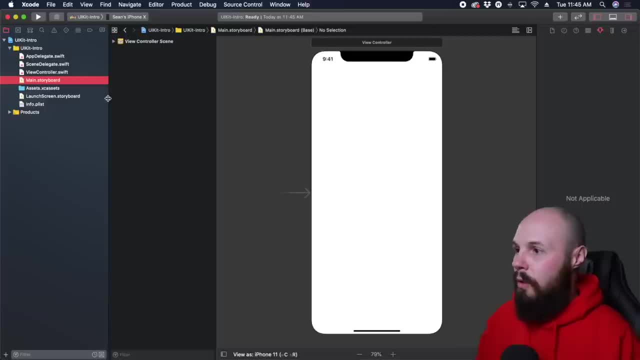 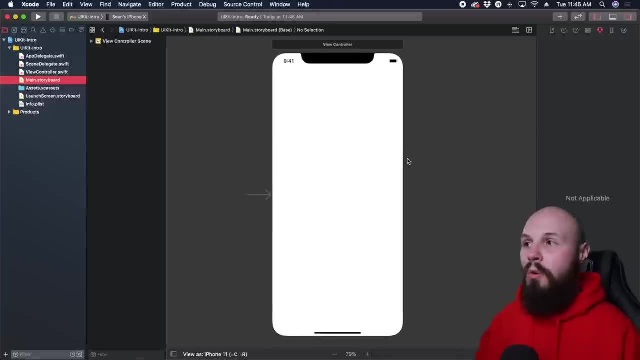 controllers are going to be entire screens, so I'm gonna make some room real quick. we're gonna drag this to the left, drag this to the left, so I have a lot of room on my storyboard here. so I just have a blank view controller, right, if we? 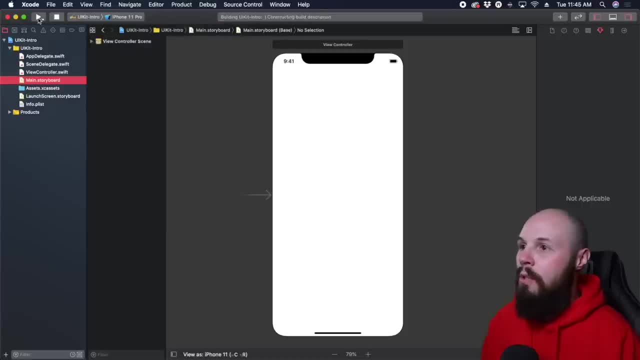 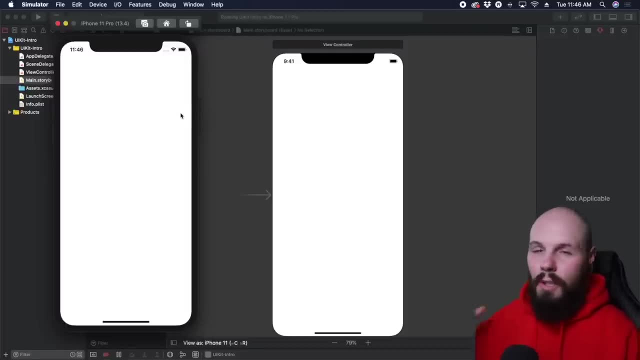 run this app, not on my iPhone X, just run it on an iPhone 11 pro. you'll see when it runs. we just have a blank white screen there you go. nothing's on there, it's blank. we're gonna fix that as we add stuff to it, but go ahead and. 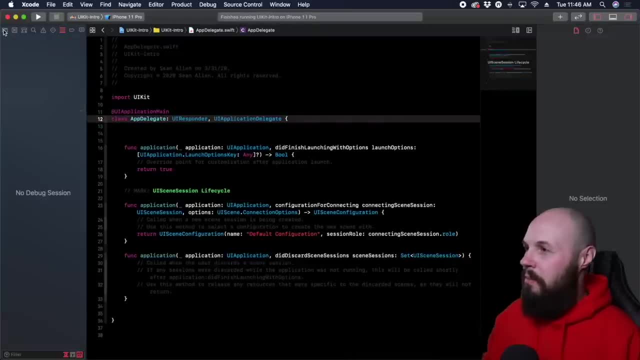 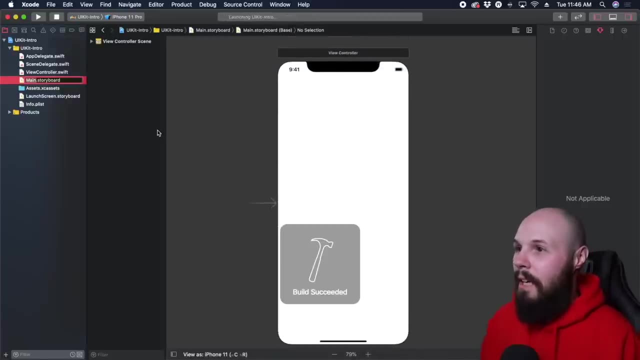 close that, stop it. oops, I closed it first. that's new in Xcode 11.4. I messed that up. I hit that little red dot up there and so if you don't see that, let me run it again. this is kind of off the cuff, because Xcode 11.4 just came out. 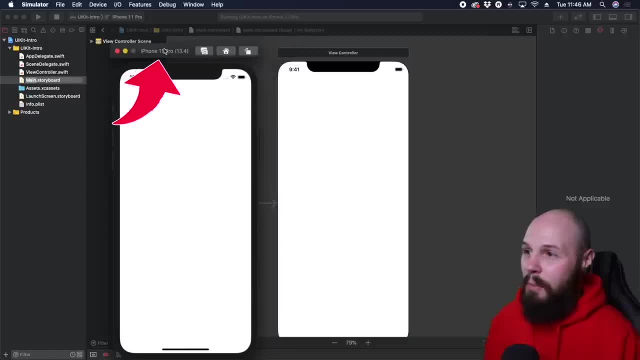 like two days ago. so now we have this toolbar above our simulator. we used to not have that prior to Xcode 11.4, so I can't see that right now, so I'm going to click on that and send it back to WPX. that's our software to get it, I guess. 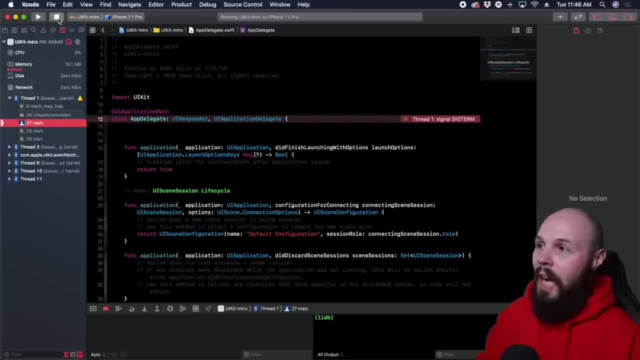 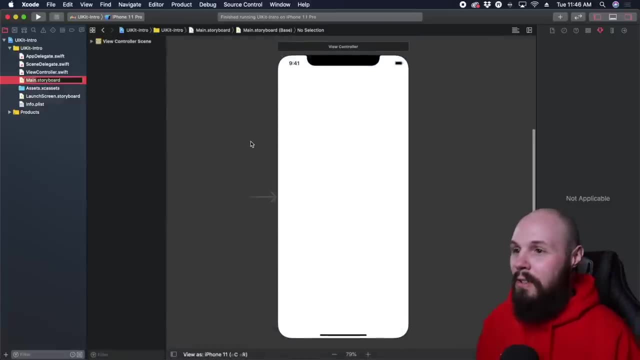 I guess- and I'm just I'm not used to using it yet- when you, when you're running your app, if you click this X, it'll like crash your app like that. so make sure you hit this stop button first before you hit that red dot again. new. 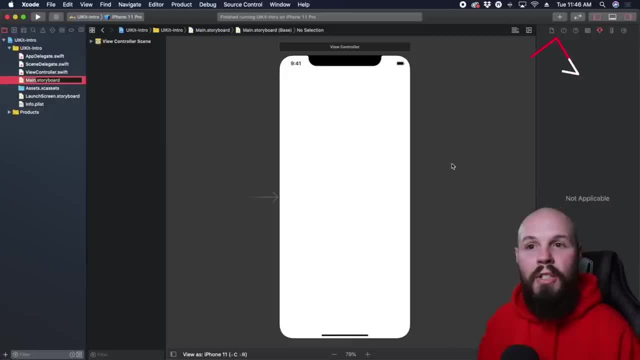 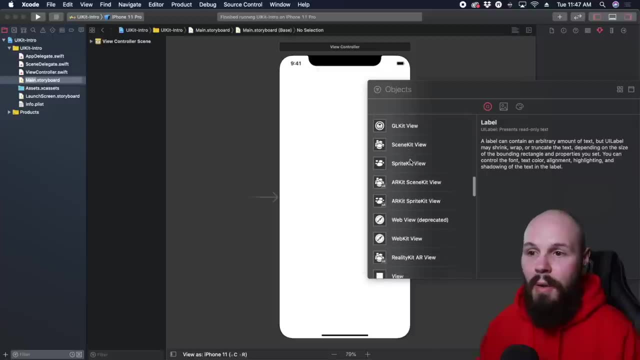 in Xcode 11.4 brand-new. so here we are in our view controller. let's start adding elements onto our screen. so the way we can do that is this plus button up here. if you click on that, you'll get a menu that you can. you know, you can see. 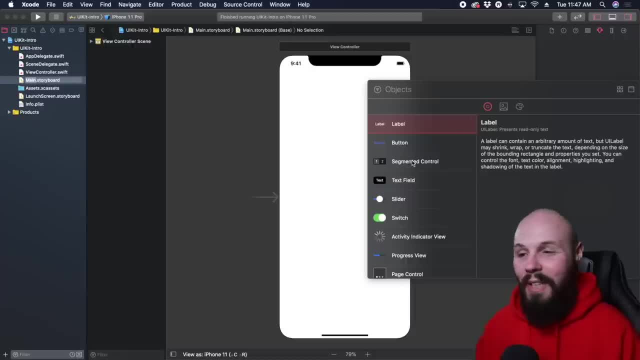 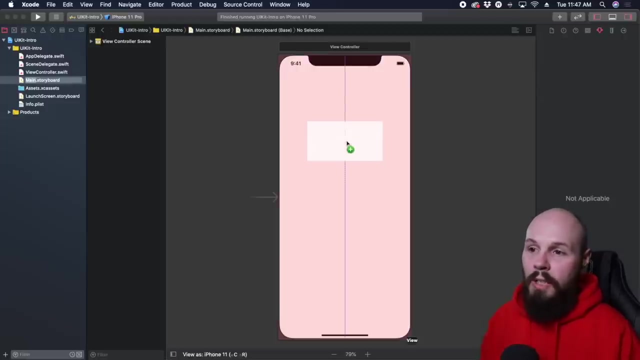 right, we're gonna start off with the basic stuff again. UI kit is very, very vast beginner course, starting off with just the core essentials here. so let's start with a view. so if you type UI view and now you'll see this view here, you just drag it onto the screen. so a view is just that, it's kind of like a. 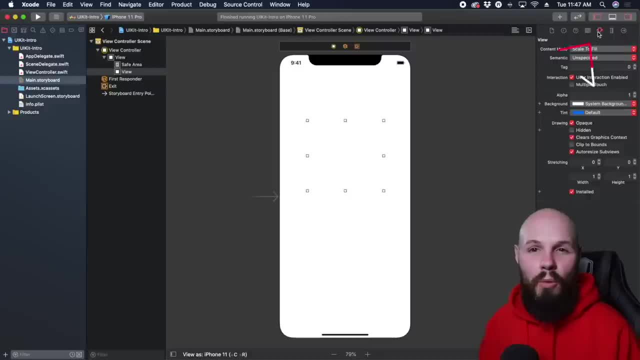 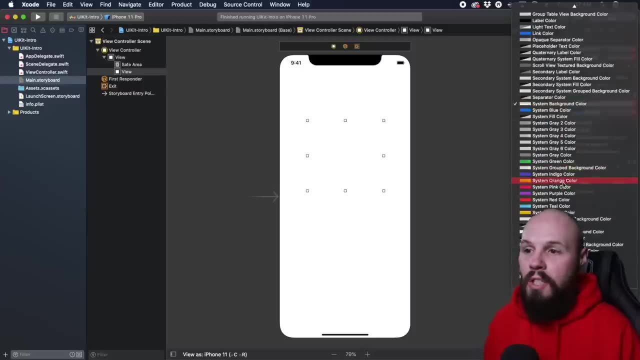 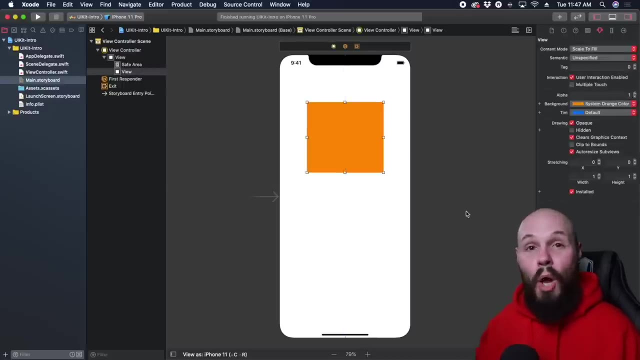 container, if you will. so we can also over here on the right in the attributes inspector see: background is system background. let's make it system orange color for our view. so boom, there you go, there's our view orange on the screen now. remember in a previous video we talked about auto layout. when you put 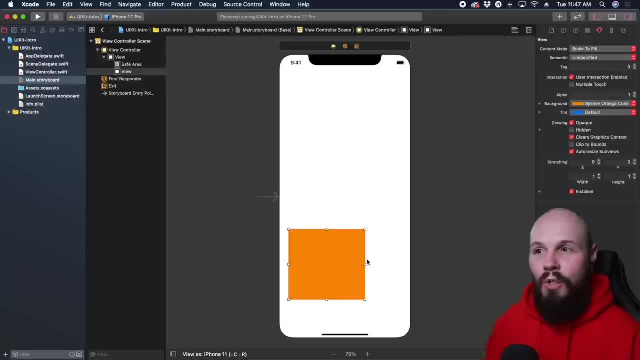 stuff on a screen like you can put it here, but it's not constrained. but because we're doing this on the iPhone 11 watch when I run this, you should see it. they're not sure. I guess we'll see what happens. I don't. I don't often build. 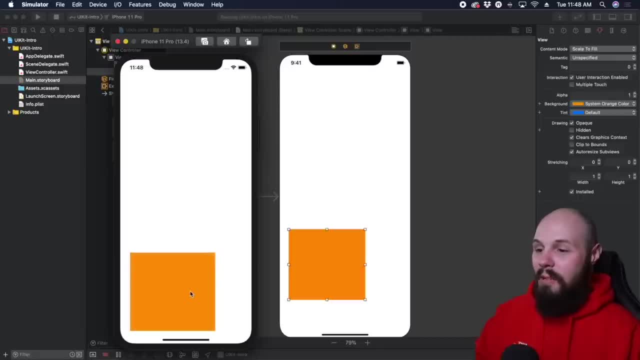 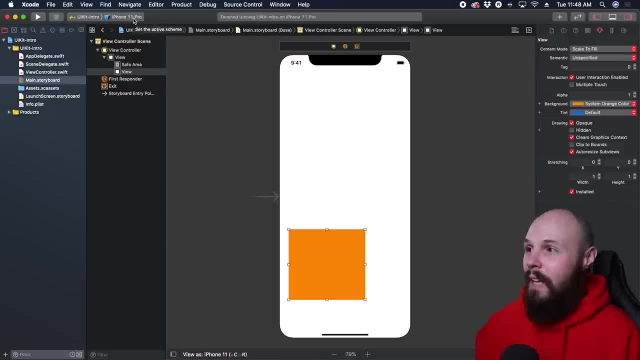 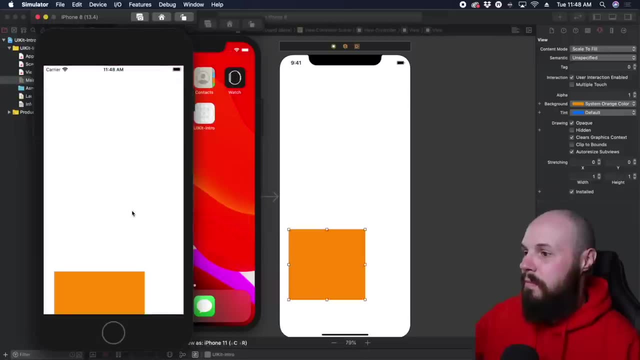 it on here, but now, without constraining something again. this is back to that auto layout. let me run it on an iPhone 8. run, you can see, because we haven't told it where to go. it's not where we want it to be, and this is where auto layout. 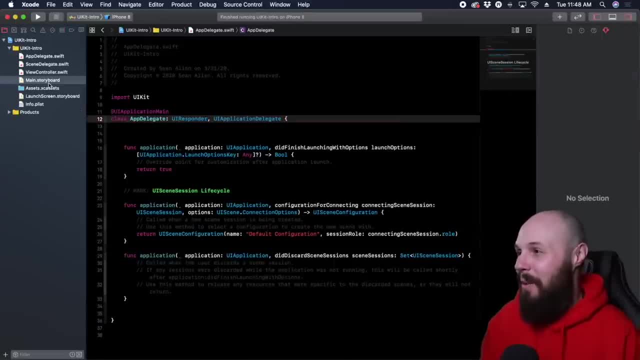 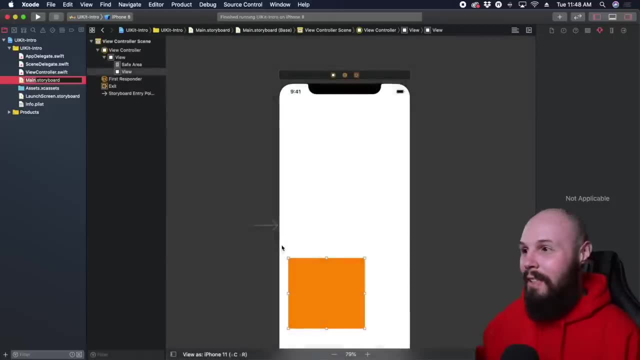 comes into play, dang it. I did it again. I'm gonna probably do that a bunch. I'm not even gonna edit it out. just to show you the pain of sometimes, when Xcode introduces new stuff and you've been using Xcode for five years. bad habits, hard to break, so alright, now let's actually constrain this view using 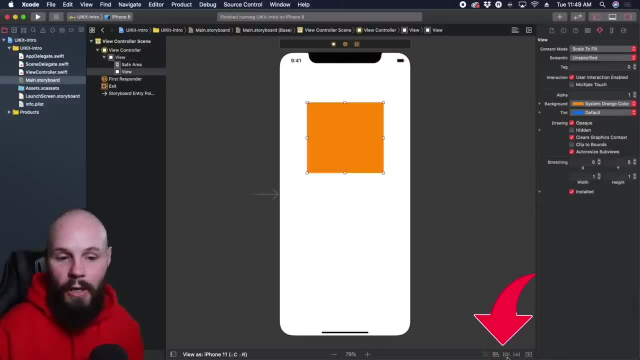 auto layout. so down here these buttons are how you set constraints. I call this one the tie fighter for obvious reasons, but let's click on the tie fighter and you can say: look, I want this to be real quick. let's explain safe area. so the safe area was new with the notch phones. if you notice how the notch comes down. 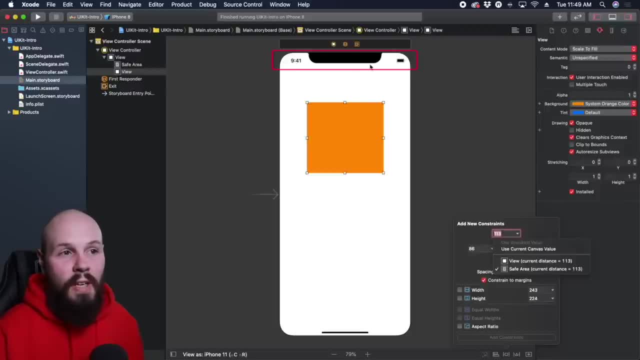 and then you have the time on the left and the battery on the right. well, the safe area is like everything above the notch in the corner if there is no going off in in the corner or on the bottom when you use the 이�. so if you pin it to the safe area, it's not going to go above the notch. and 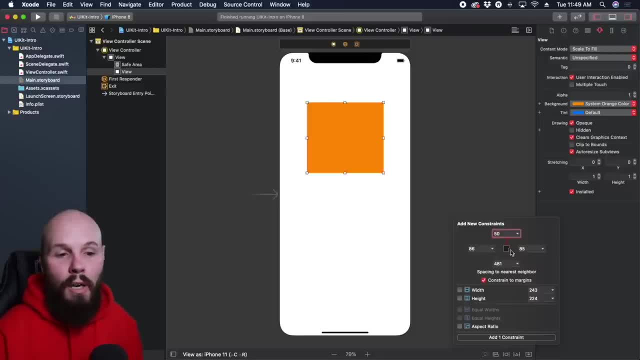 look weird. so we will use safe area. so we want to pin it. let's say 50 points- remember points, not pixels- from the top of the phone. so if you hit add one constraint now you'll see that added it, but it shows up in red. a rule of thumb. 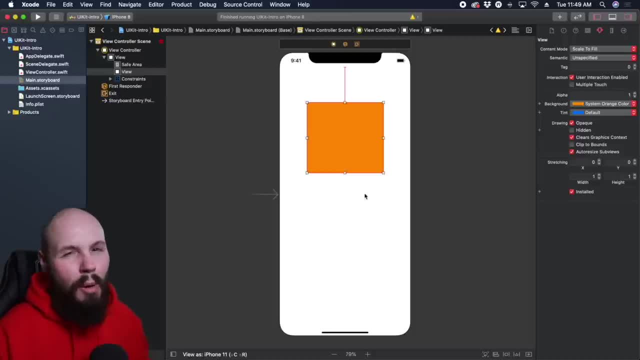 is that an item should have four constraints. if you find yourself having seven constraints on one item- height, don't worry about that again. the rule of thumb: four constraints. so let's set those four constraints because you need to give it a height, a width, an x coordinate and a y coordinate. those 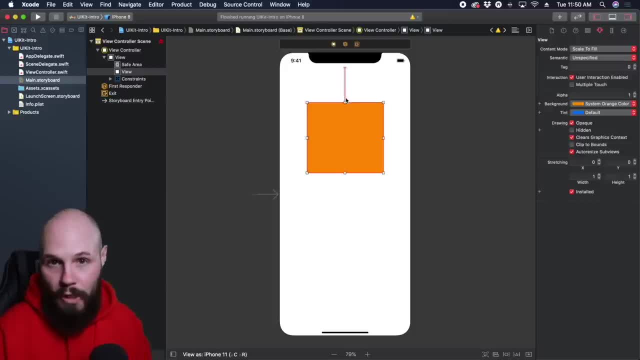 are typically the four constraints you need. so we gave it a y coordinate, right, because we told it 50 points from the top of the safe area. so now let's go back here. let's give it a height and width. we want to make it 200 by 200, so that's our height width. now we need to give it an x. 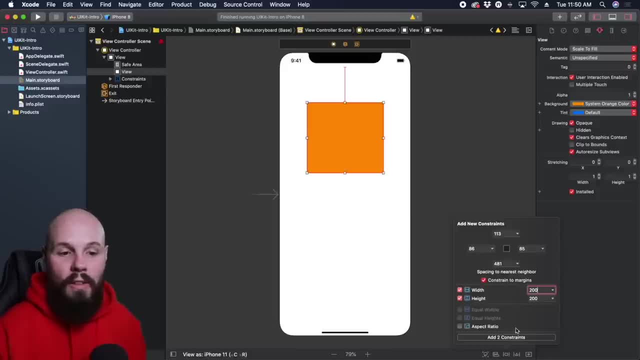 coordinate right, horizontal. well, we're going to center that. well, you can't do that in this menu here, so add two constraints, all right, so it's still red. we're almost there in these little, two little bars to the left of the tie fighter called a line. that is where you get, you see, horizontally. 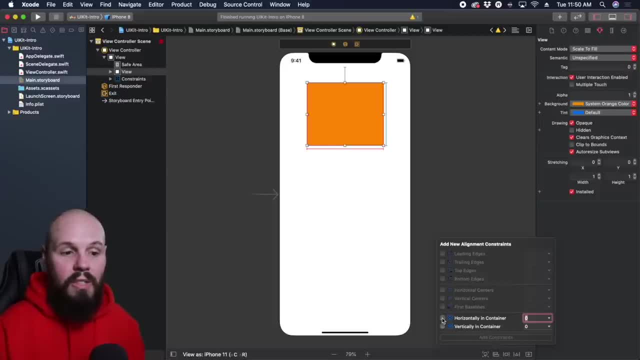 center in container and vertically center in container. so we want to center this horizontally, so we click on that: add a constraint. now we're all blue, everything's good. we have our four constraints on this. so now what we're telling auto layout is that this is always going to be 50. 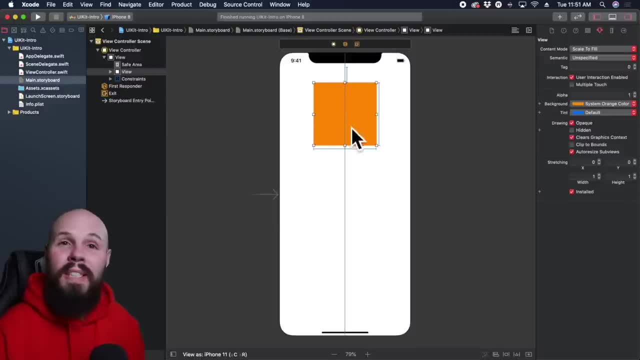 points from the top of the screen, no matter how high we want it to be. so we're going to center it and it's always going to be 200 by 200. so again, whether i run it on the iphone 11 pro max, we're going to go with the biggest phone size. okay, there it is. 50 points from the top and then 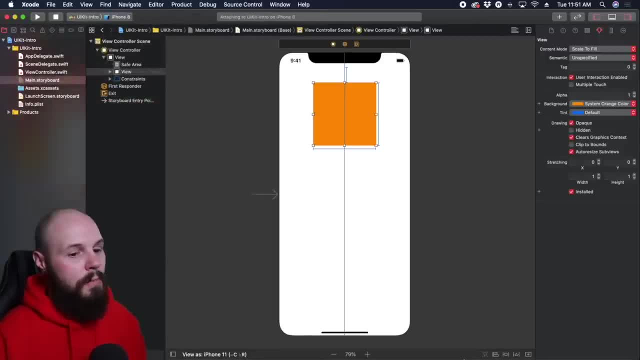 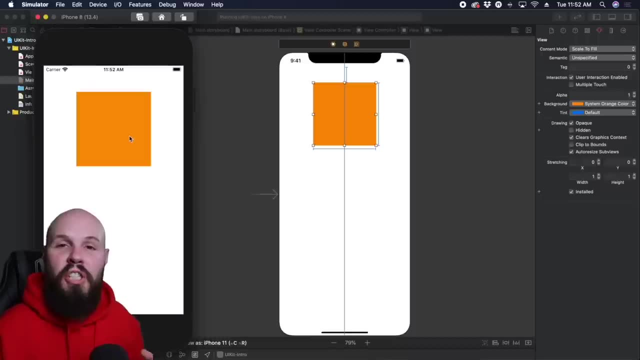 the same thing. uh, if we stop it, run it on the iphone 8. i've got to go to our simulator. oh, there it is again, 50 points from the top centered. so that is what auto layout does. it helps you position your elements no matter what screen size. and actually you know what? uh, i'm not seeing the 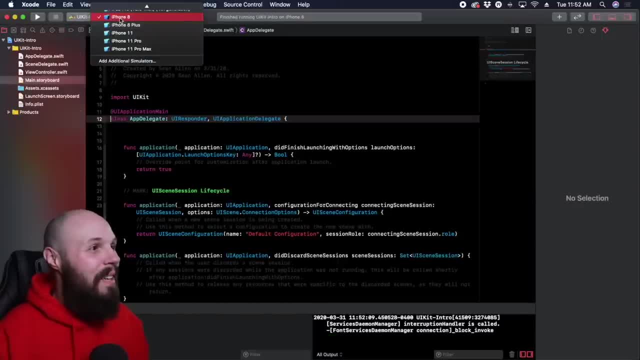 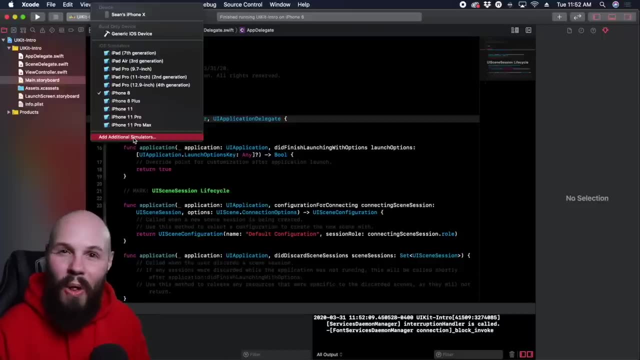 iphone se, dang it. i keep doing that, leaving it in um. the iphone se, uh, isn't on here so we can add additional simulators, as you see, because the iphone se is that small iphone 5 screen size, at least as of now. allegedly, the iphone 9 is going. 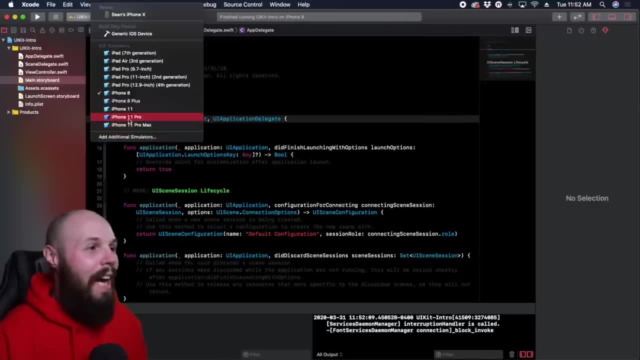 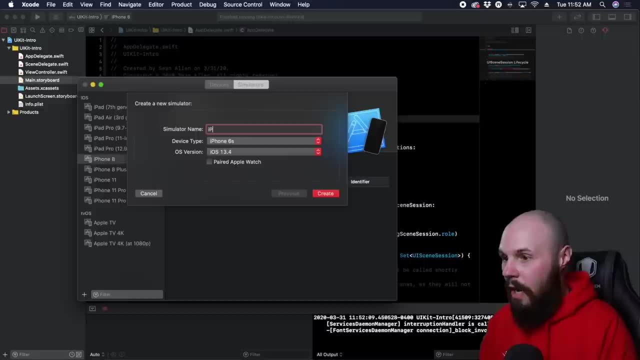 to come out and replace the iphone se but the small iphone 5 screen size so you can hit add additional simulators. and then you hit this little plus button on the left and so the simulator name iphone se and then here's where you can any simulator you want watch. when i click this, 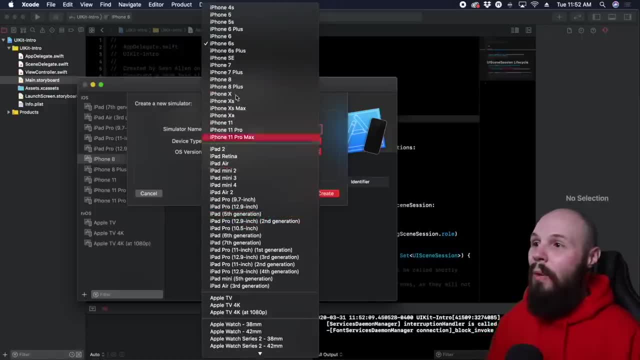 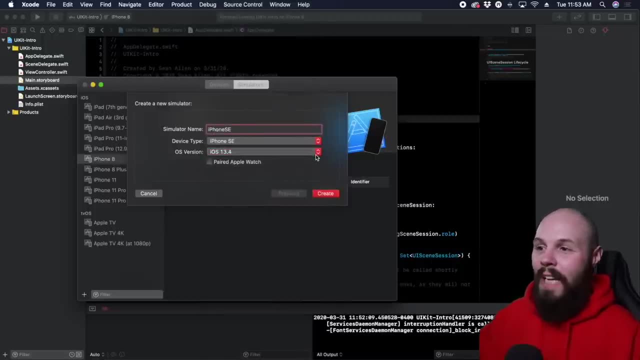 oh man, a whole whole bunch of simulators. and then you hit this little plus button on the left. which of devices you can add. we want to add the iphone se, because, again, that's that little iphone 5 screen size. you can even specify an ios version. um, you have to download more simulators, but i 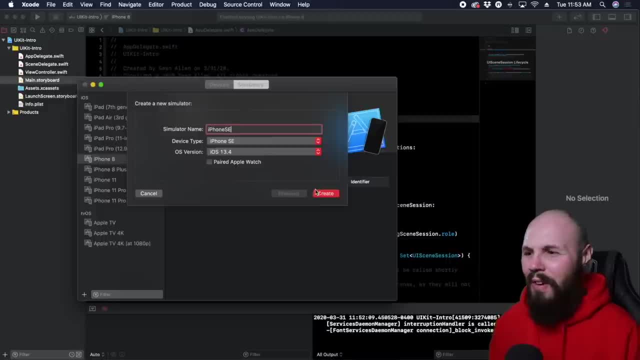 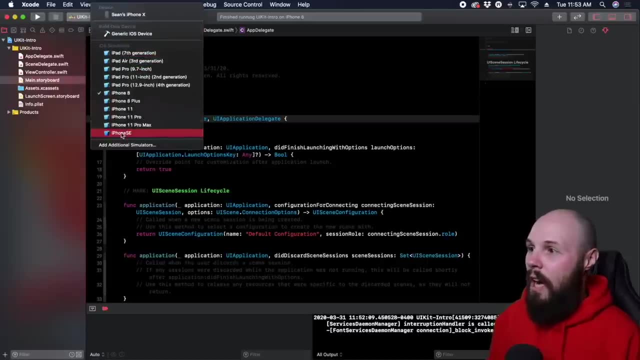 wouldn't mess with that. now that's pretty advanced, you know. if you want a specific version of ios to test again, so hit create and then now we have the iphone se simulator. so now you see, iphone se pops up here. so now we click on that and now let's run it. this is a way to test. you know, ui on various 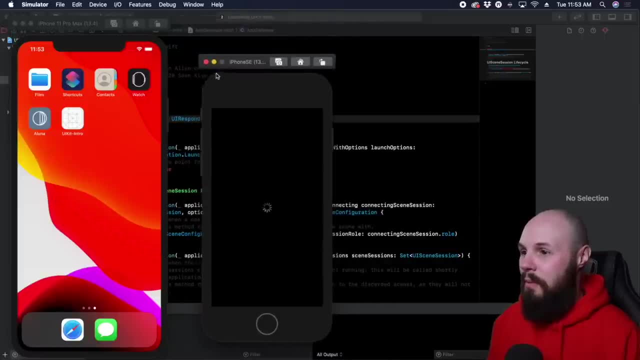 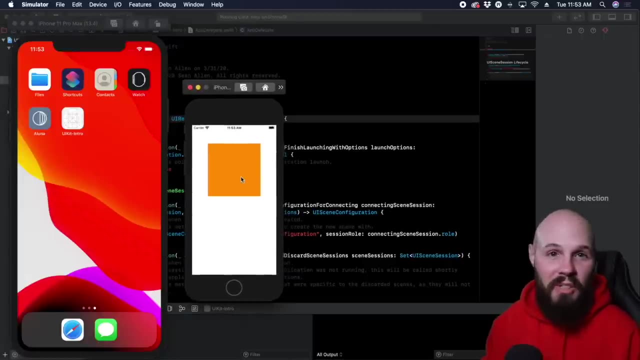 devices. you can see the small iphone se. well, it's not small, it's actually huge. let's make it. make it how it would actually look next to the old iphone 11 pro. but you see we're 50 points from the top, uh, centered horizontally 200 by 200, and i can run this app here, you can see. so that is what auto. 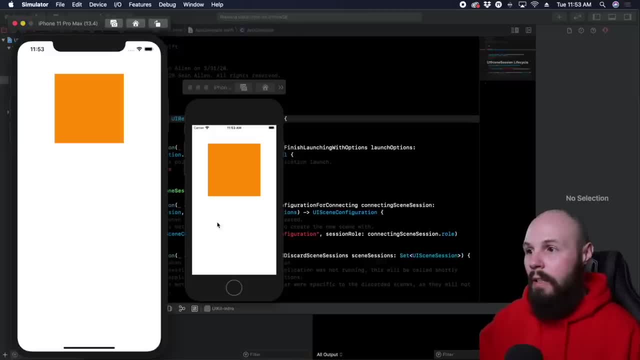 layout does again. you tell it how to position itself and it works on all the screen sizes. now, that was a super easy example. we're going to continue adding elements onto the screen to show you other ways to use it, so let's go ahead and stop our simulators. 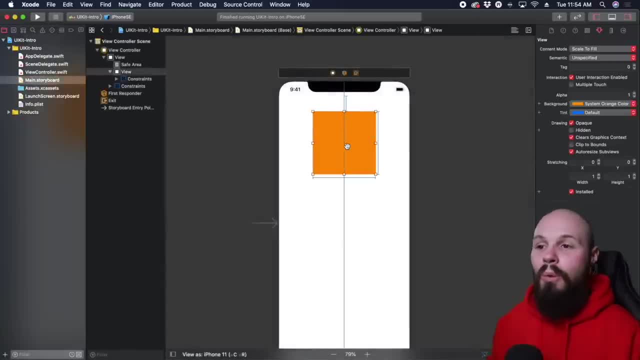 and back to mainstoryboard. so that is a ui view. uh, ui view can just be this a shape, but you can also, like put stuff into a ui view. uh, let's say, let's actually grab a label so you can either hit this plus button or what i've gotten used to doing is do command, shift, l, and that'll pull this up. 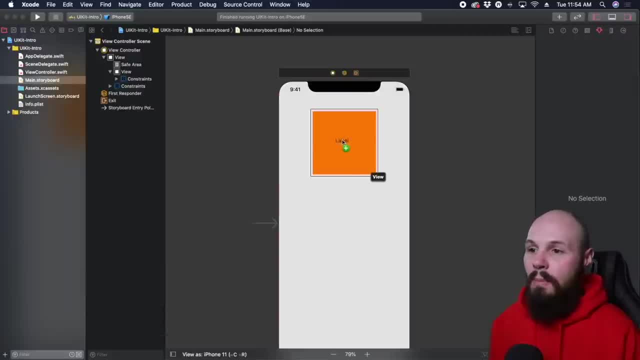 command shift l. so let's put a label. except now we're gonna put the label inside the ui view so, again, you can have a view that holds other views. and, by the way, ui button, ui label are all sub classes of the ui view, so you can have a view that holds other views. and, by the way, ui button. 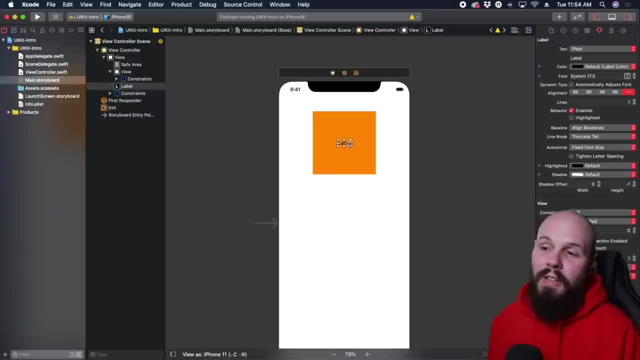 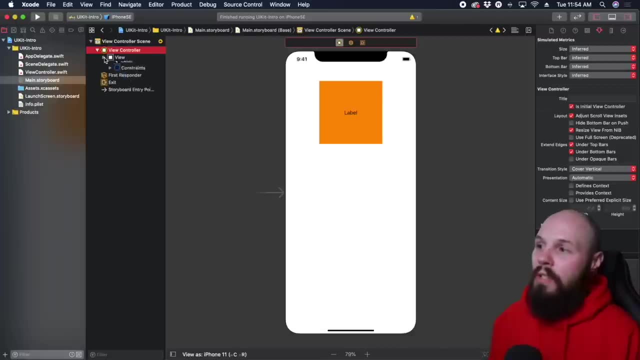 of ui view. so now we can actually constrain this label within this ui view. and over here on the left you see your view hierarchy so you can see if i minimize my uh. well, this is the overall. a view controller comes with a big ui view that covers up the whole screen. but you see we added this ui view. 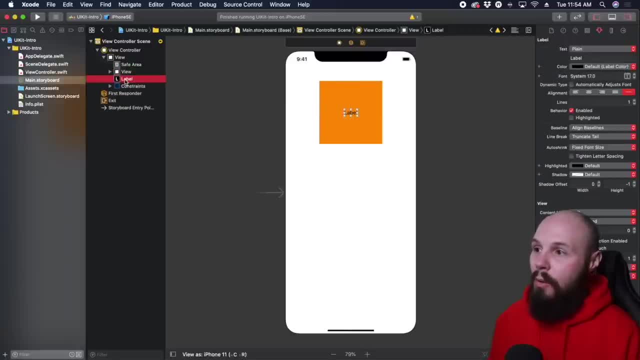 here and you see within that ui view, uh, we have a label. well, that label's not actually in the ui view. drag it up here now. the label is in the ui view. so you can use this view. hierarchy on the left to. you know, put stuff within each other to. you can use this view hierarchy on the left to. you know, put stuff within each other to. 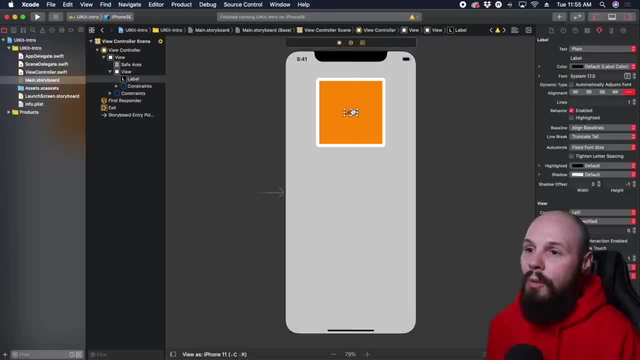 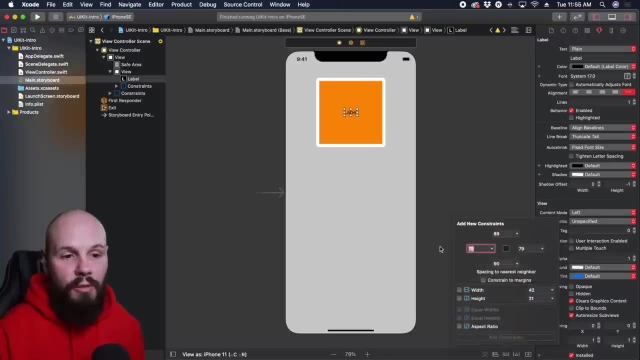 you know, build your ui. but now that we have this label within the view, we can constrain it inside the view. so let's say we wanted our view- click the tie fighter- to be pinned to the left of the container view of the view. so zero, zero and hit, add two constraints. you're going to see it stretch. 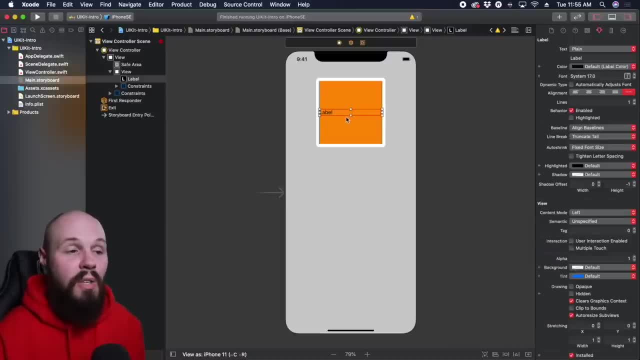 out right. it's stretched out to fit the uh to the edges of the view. and let's say we wanted it to be pinned to the top. let's say zero again to the top of the view. add one constraint. you see it move up. and remember i said labels don't need a height, they have intrinsic content size. 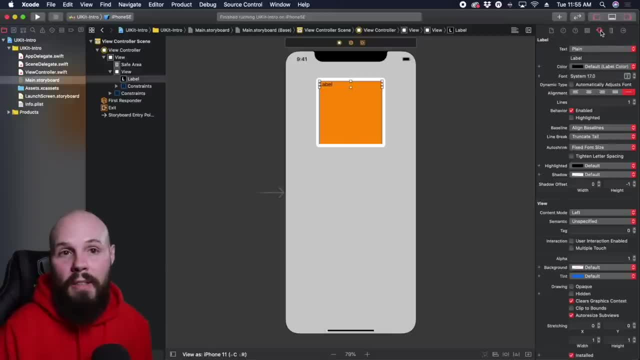 you know, based on how big the label is. but and then over here on the right, the identity inspector here, attributes inspector, we can name this, you know, orange, right, we're just naming, uh, our square here, so we just constrain this to the upper right. uh, within this view, to show you how you can have. 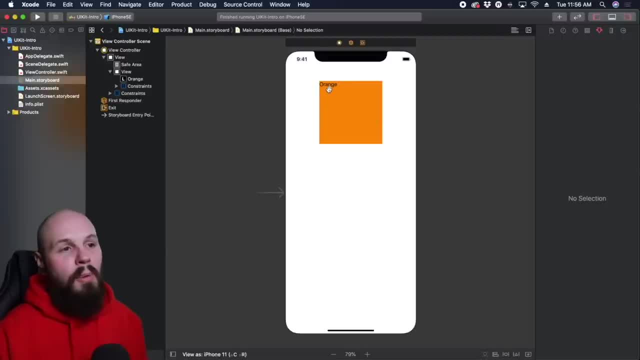 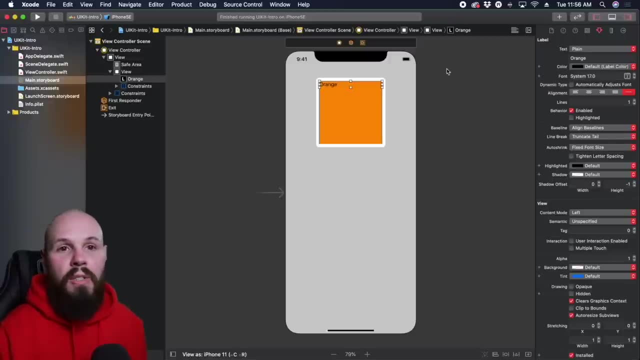 you know views inside of views, but you know that kind of looks weird upper right. let's say we wanted that centered. well, we already have constraints set, so the answer isn't to just set more constraints. uh, the answer is to hit this ruler button to the right of the inspector here. 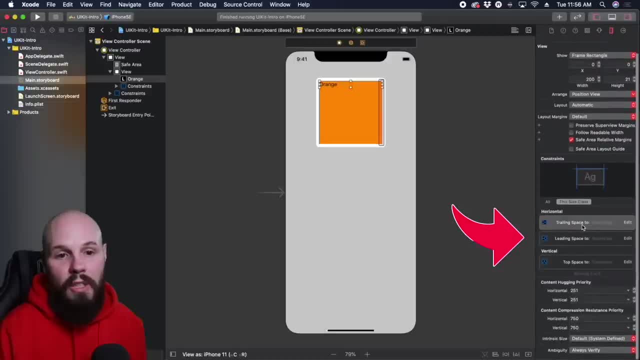 size inspector, and you can see down here. we have constraints: trailing space to super view, leading space to super view and top space to super view. super view is the view that it's in, by the way, right, we put it in this orange view. that is the super view. so what we can do is you can just click. 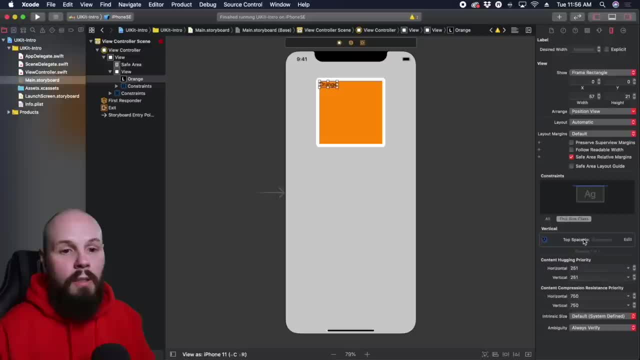 on those and delete right. we don't want it to be, uh, constrained like that, so we delete all our constraints. now let's come back to the alignment constraint and let's just vertically and horizontally center this in the container. so there you go, there's our label, just vertically. 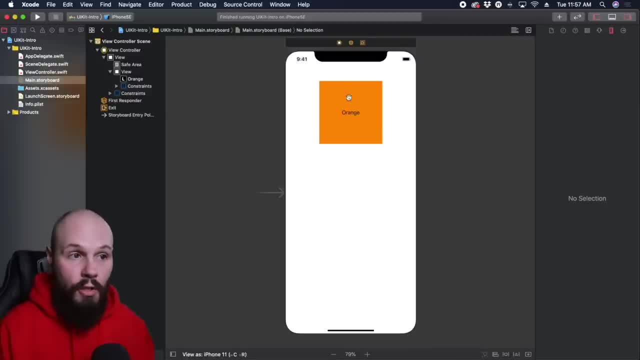 now, if it was outside of this orange view, the container would be the view on the screen, so it would be in the center of the screen. but because we're inside the orange view, the label orange is centered in there. so now let's explore some other ui elements here. command shift l- let's talk. 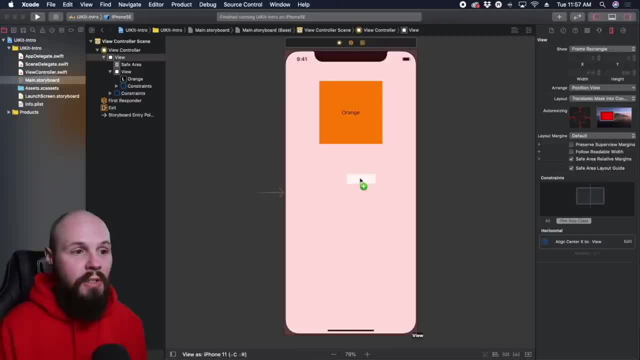 about the text field. so if you want to enter text, grab a text field, pull it here and now you can see we get this. uh, it's not very wide. well, if you remember the example i gave for model layout, where i had a text field that was straight across and then you just slide it down to the bottom of the 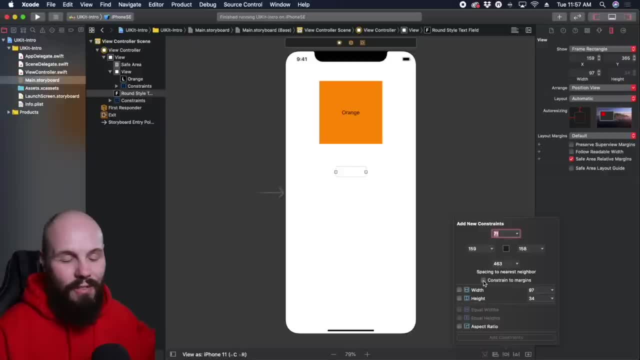 text field and you can see it's a little bit more rounded. now, as we go along, we want to get a little bit more of that padding of 30 on the left and 30 on the right. that's how we do that, so click on the. 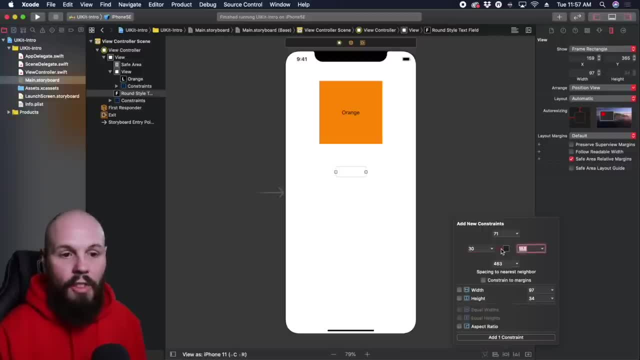 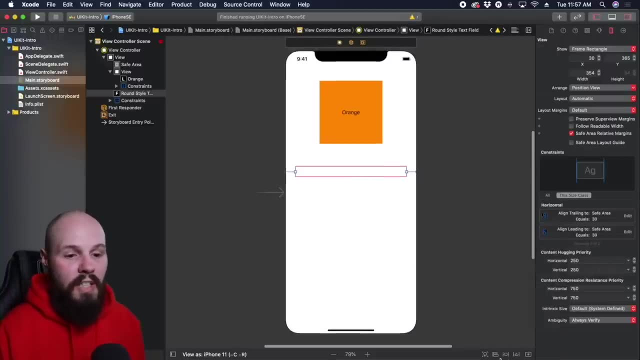 tie fighter. we want to. we don't want to constrain a margin that'll give us default margins. we don't want to do that. we want to add our own. so safe area- cool, do not zero 30. and then same thing over here: 30 for the right hit, add to constraints, and now you see that text field stretch. so there's. 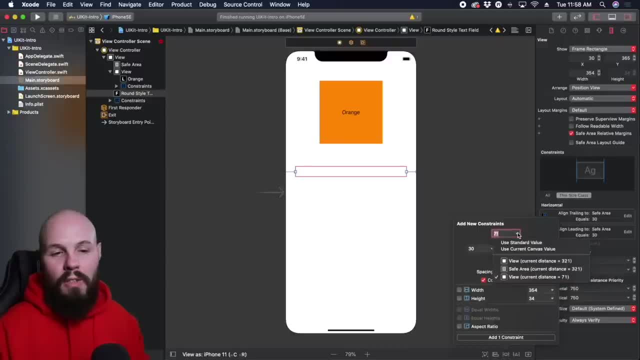 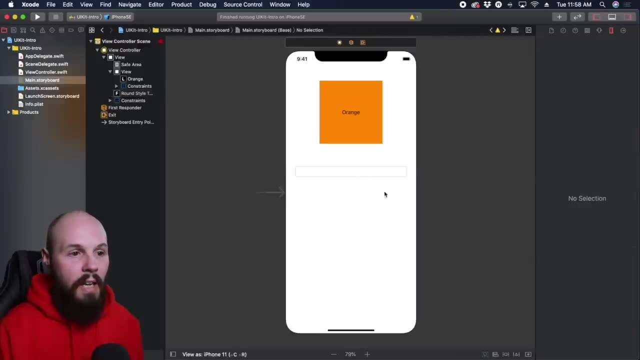 the orange view, which again is this view right here. I know that's confusing because there's two views, but you can see current distance is 71, it's closer. You can also do constraints like this. Let's not add that. 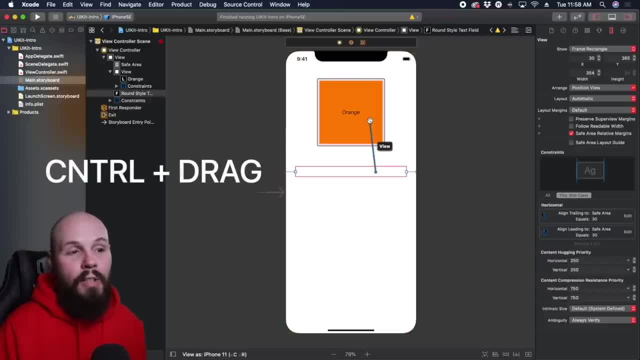 If you click on the element you can control and drag to that view, And then now you can get some constraints here. So we want vertical spacing. So bam, now a vertical space. So there's a couple of different ways to set constraints. 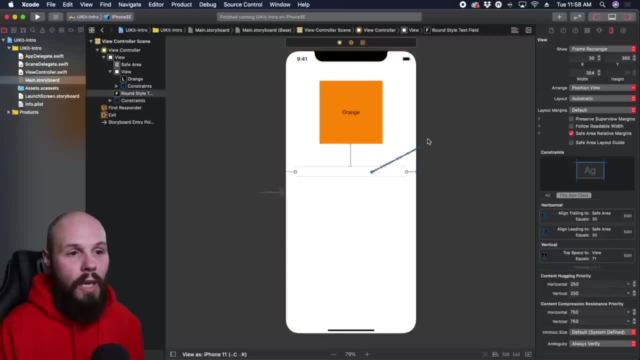 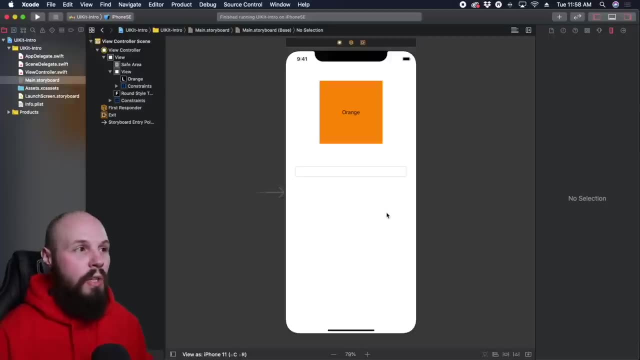 the TIE fighter view, and then also again control drag to whatever you want to constrain it to. But now let's take a look at this in action. You can see it on the iPhone 11, right, It stretches out to the edges of the screen with 30 padding. 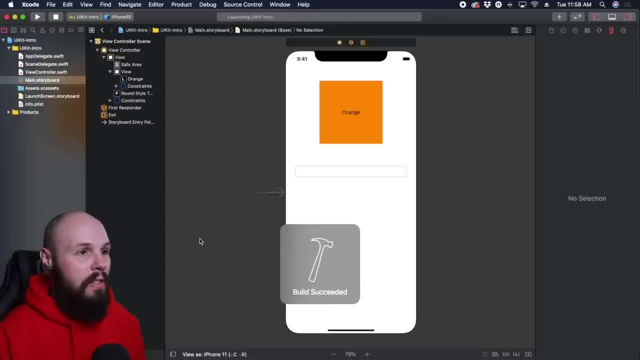 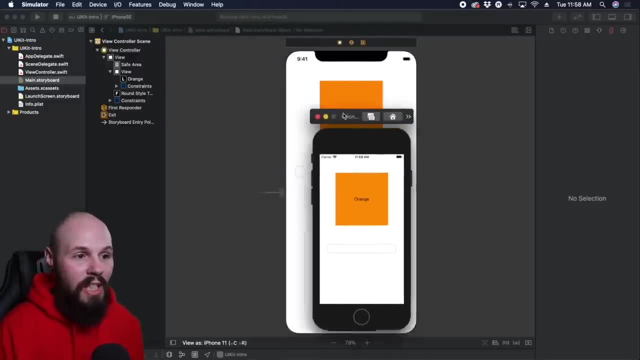 Again, let's run it on the iPhone SE, because that's not as wide as the iPhone 11.. And you can see it still gives us that 30 padding on the right and the left, but it's you know, it's a much skinnier text field, as you can see. 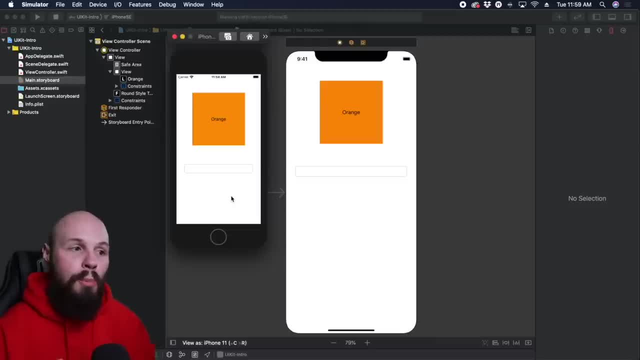 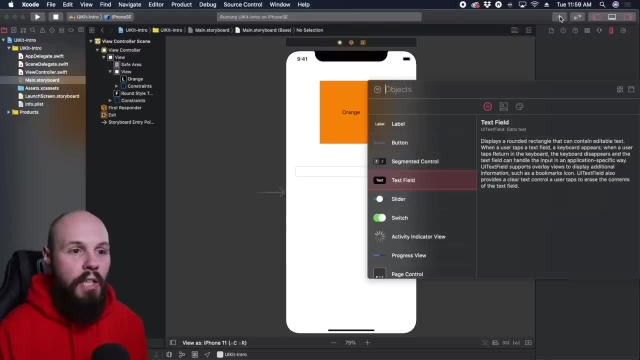 because, again, the screen is wider. So you can see how auto layout helps us adapt our UI elements again to the various different screen sizes. And for practice, let's add one more element here, Let's add a UI button. So again, 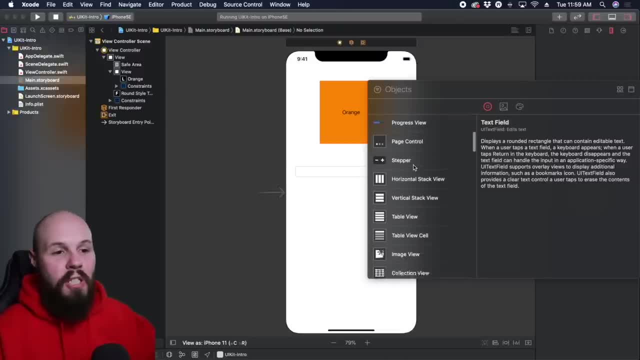 label button segment to control slider switch. There's so much here in UIKit: Image view that holds images collection view, table view. I'll talk about that in a second. Again a lot to do in UIKit. We're going just the fundamentals here. 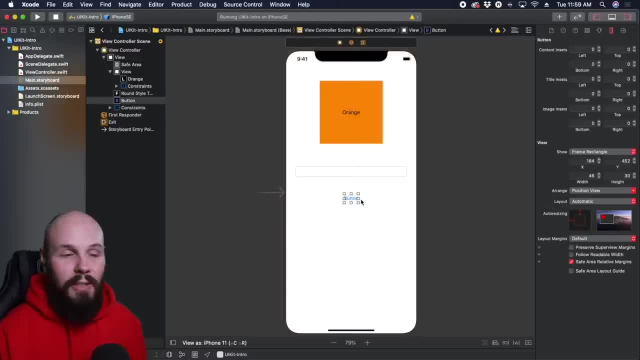 So now a button. a button does again what you would think a button does. Whatever action you want to attach to the button being tapped, that's what you do. Let's actually pin this one to the bottom here. So again, I'm going to open up my little TIE fighter. 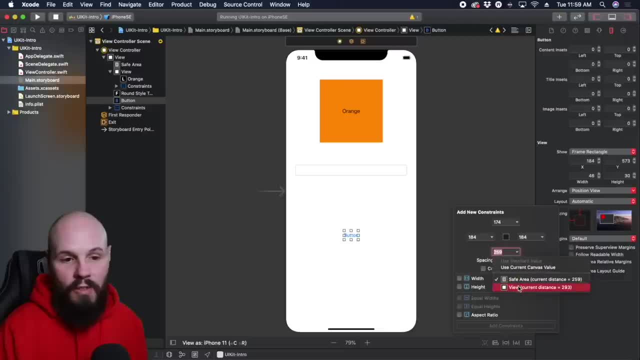 and not constrain the margin. So to the bottom here. we want the bottom of the safe area. Let's do 40 points from the bottom And we want this to be, let's say, a width of like 250.. It's good for a button. 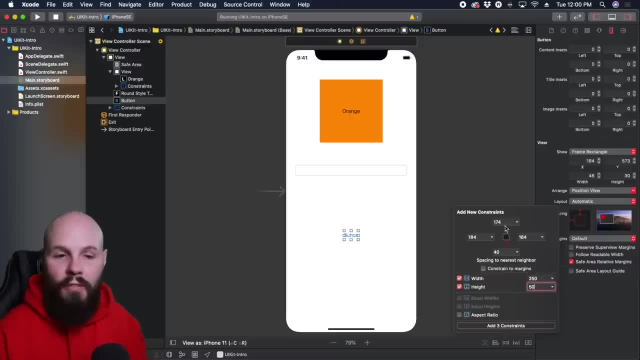 And we want our button height to be 50.. So again, we got our height and width. We're pinning it 40 to the bottom, So let's add those three constraints. There it goes. Now it needs to know where it is horizontally. 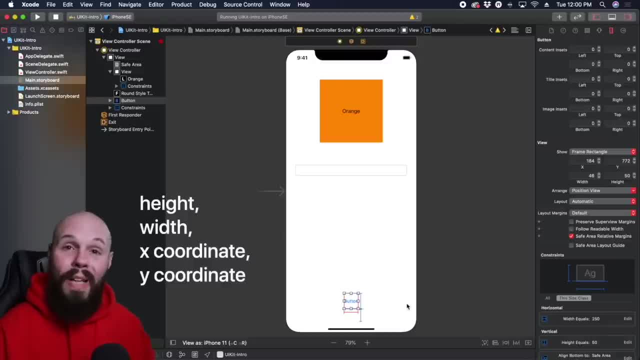 Again, height with X and Y coordinates. That's what auto layout needs to know in order to place it, Those four pieces of information. So our button knows its height and width right. We hard-coded that. essentially, It knows where it needs to be vertically. 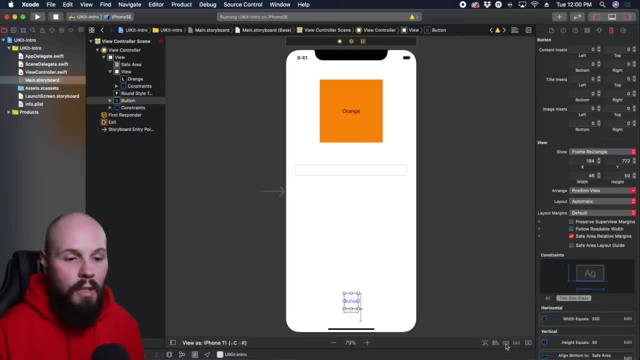 We said what? 40 points from the bottom. Now it needs to know where to be horizontally. So we're going to say horizontally, center in container. Add one constraint. So there's our button. Now back to the attribute inspector. Let's start customizing our button a little bit. 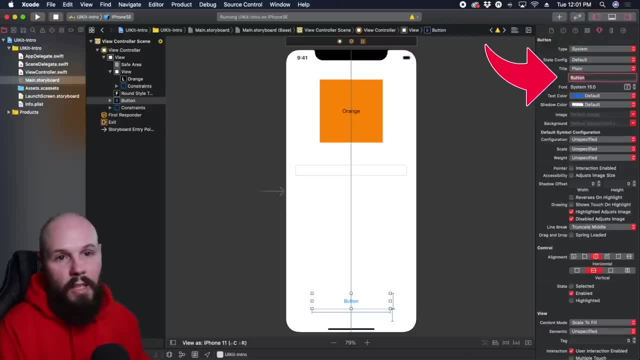 You can see all the options we have. We don't want it to say button, We want it to say this does nothing because we haven't hooked up an action to it yet. Well, now we get that blue kind of default ugly looking button. 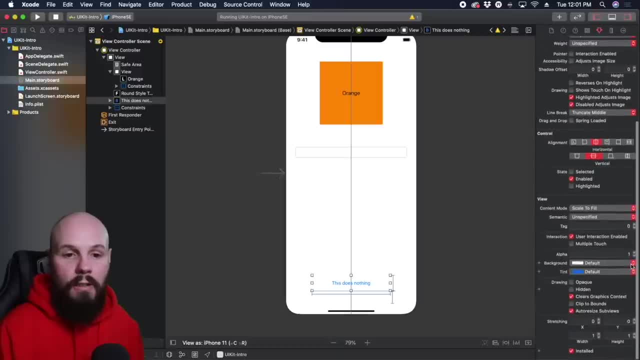 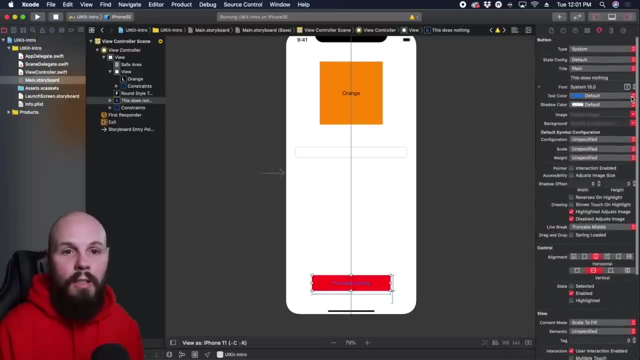 Let's change that. Let's say our background color down here we want to make system red. red button: Well, now that we have a red button, we don't want that blue font. So up here text color: let's make it white. 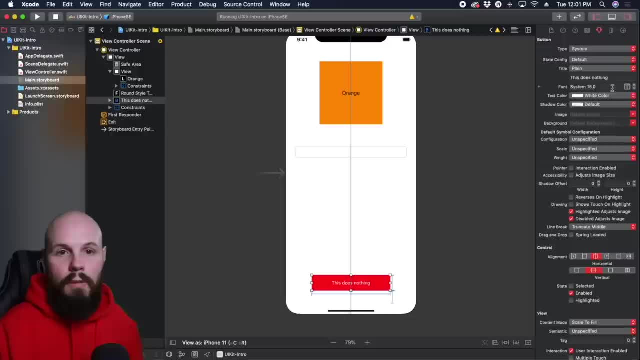 So we have white. Okay, We can customize even further The system font. we'll keep it system font, but we'll make it bold, right, And then we'll make it 22 points So you can see how big it is done. 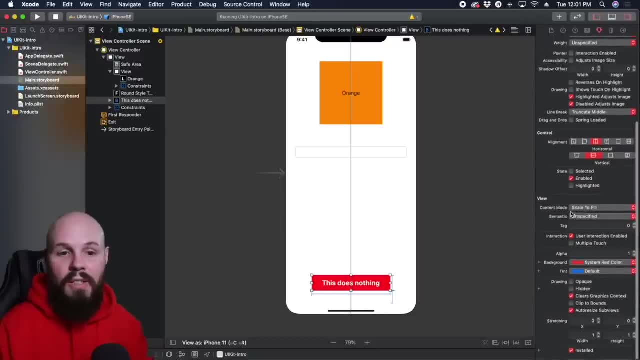 You can see, you can add an image to a button. So there's a lot of stuff that you can do to customize this button. but here you go. Let's actually run our app now. We'll keep running it on the iPhone SE. 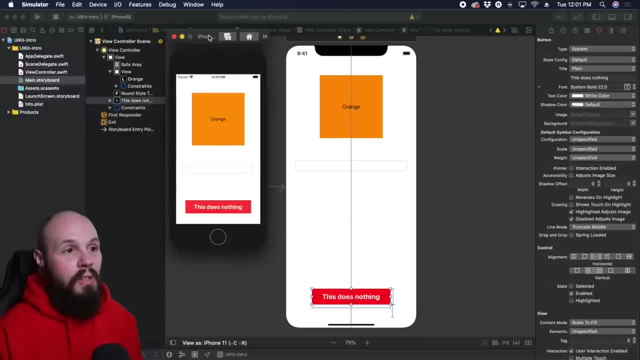 because you can see what it'll basically look like on the iPhone 11, right. You see the difference in the screen size. Look at the gap between the text field and the button- Really really large on an iPhone 11 Pro, right. 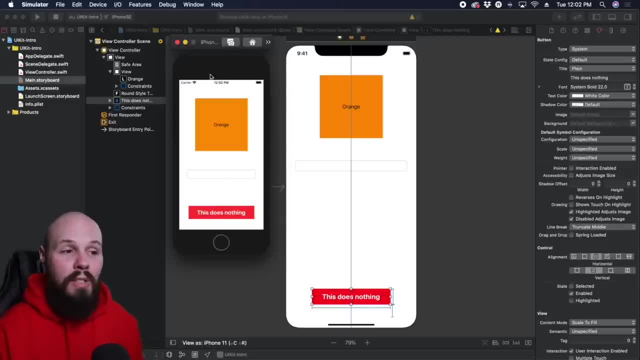 The new notch phones. You can see how small that gap is on the iPhone SE And this is a good demonstration. You know, sometimes you'll be designing an app or your designer will design an app and they'll design it for the iPhone 11 Pro, right. 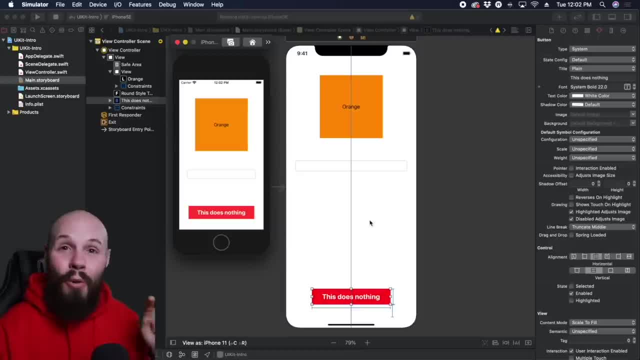 That's the new phone, That's what a lot of people have. However, converting that design with all that space to the iPhone SE, where you don't have- you got like half of that space- is very, very difficult And, like I said, auto layout can do a lot of the work. 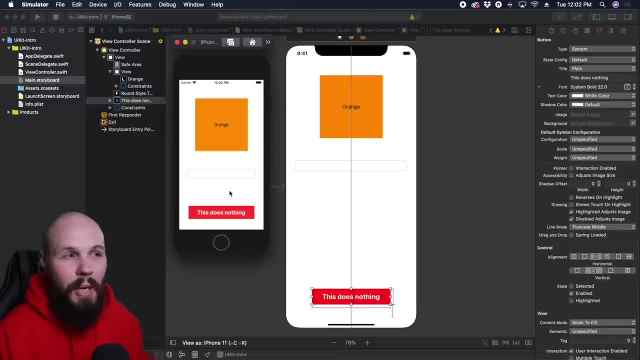 for you, but oftentimes you'll have to go in there and tweak stuff, especially for this iPhone SE. This is like the bane of developers' existence in modern day: app development. As you can see, not a lot of space that you get on the iPhone 11 Pro. 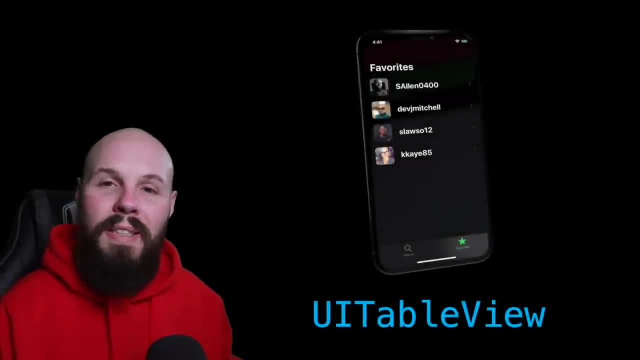 So the last couple of common ones are a table view. We'll be building a table view and a future app, but for now I'll just show it to you, cause that's a whole tutorial just to build that A collection view as well. 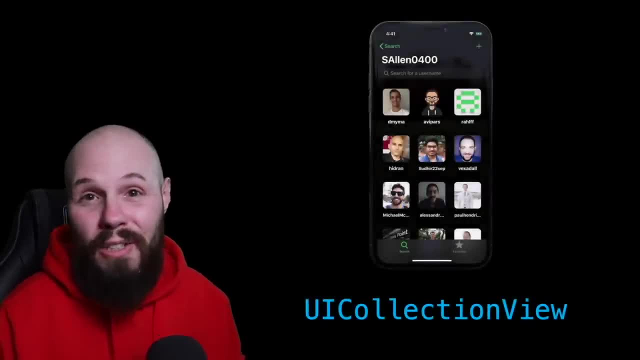 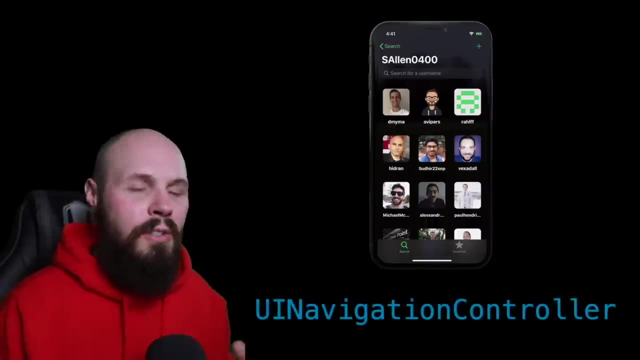 If you've seen like a grid of things like you see on this app, that is called a collection view. Also here on this app, the tab bar at the bottom, that's a UI tab bar controller. That's part of UI kit. 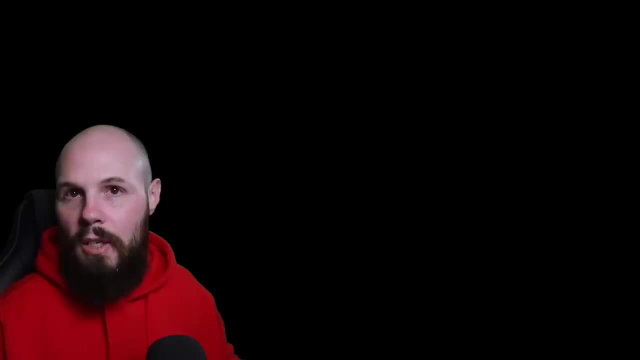 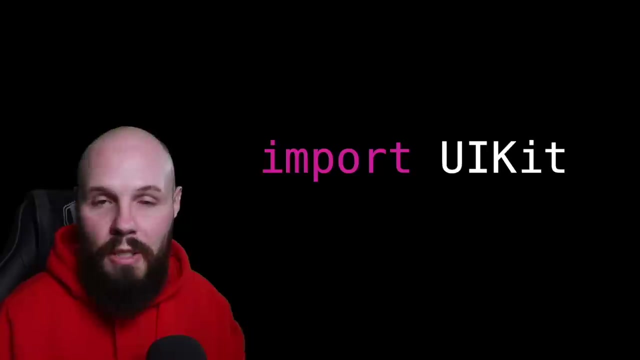 There's UI navigation controller. we're gonna touch on in an app we build. So this was just your introduction into the elements of UI kits. We're gonna be using UI kit extensively as we build our future apps in this course. So again, just an introduction. 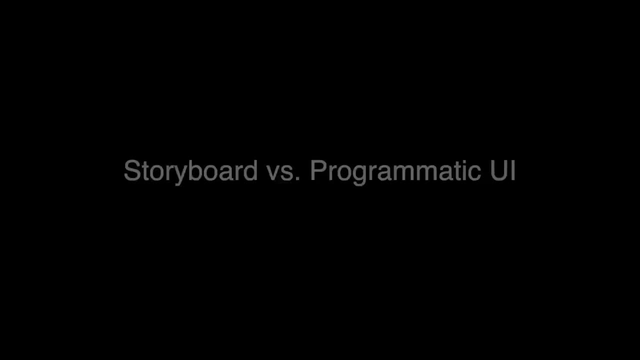 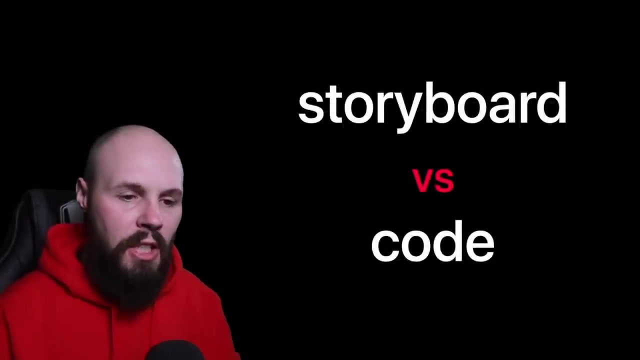 You'll get plenty of practice with the basic elements in future videos. So we just dabbled a little bit in storyboard, gave you a super basic introduction. Let's talk about like: should you build your app using storyboard How you saw with? you know it's nice and visual. 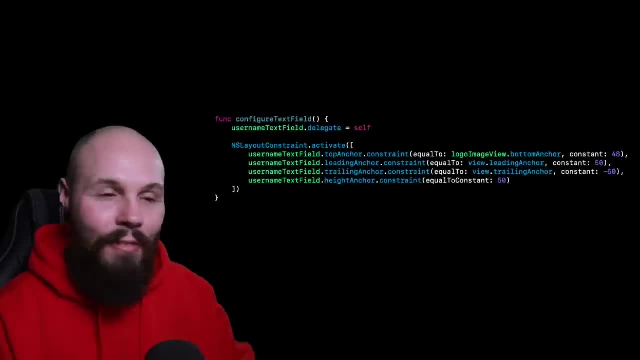 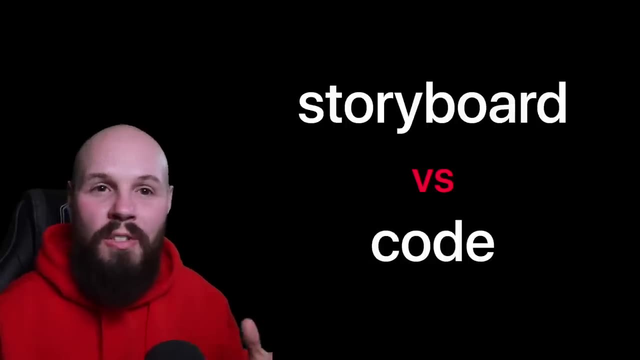 everything's laid out, Or should you build everything in code? where you have no visuals, you're just coding everything. That's a hotly debated topic in the iOS developer world, but I'm gonna tell you the pros and cons of both And then later in the course when we build our apps. 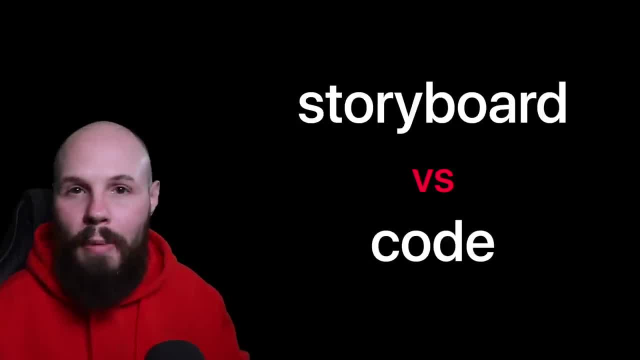 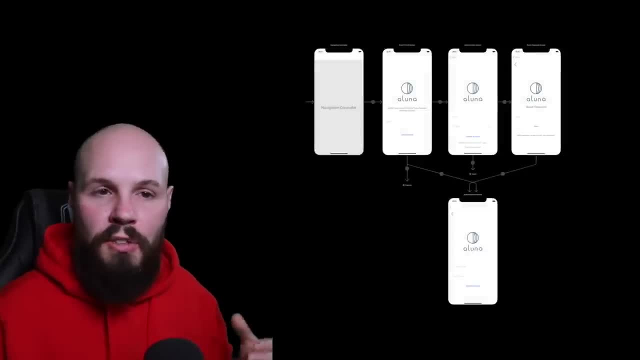 you'll get a little taste of building it via storyboard and building it programmatically, And then hopefully you can start to form your own opinion on the debate. So let's start with storyboards. A lot of the benefits of storyboards are again: 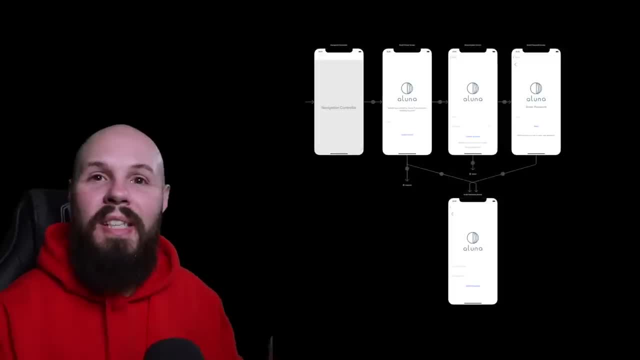 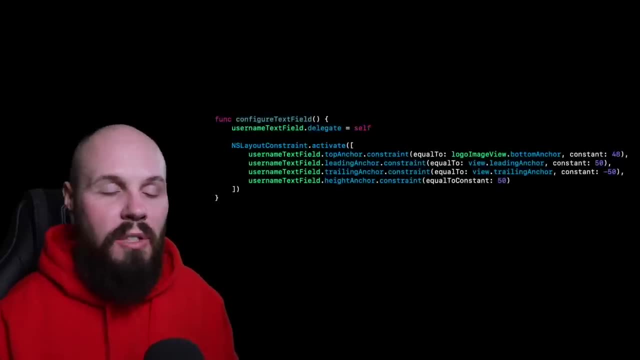 the visual layout that you see here, right? It's nice to see how your app interacts when everything's laid out for you, And it actually hides a lot of UI code right? Here's an example of just laying out one element programmatically. 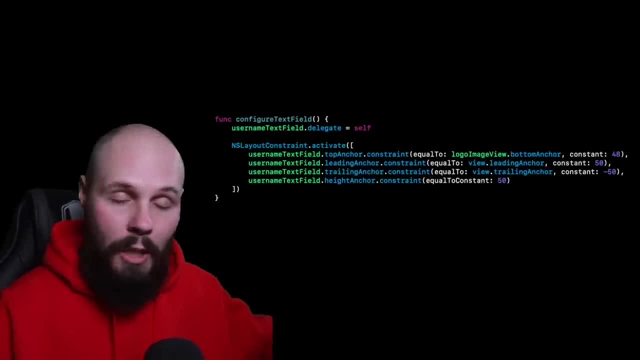 And you can see there's four lines of code to set the four constraints. Remember we talked about typically you need four constraints. Remember we talked about typically you need four constraints. Well, imagine laying out a whole screen that has a bunch of elements on it. 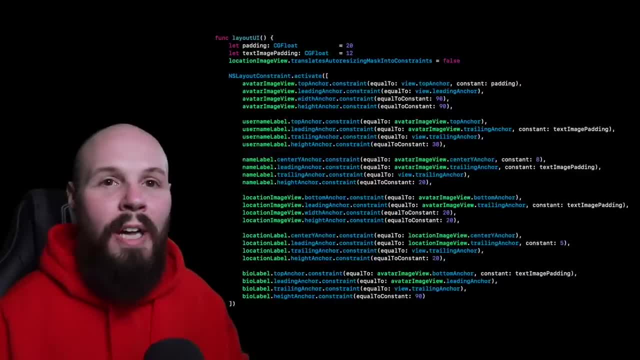 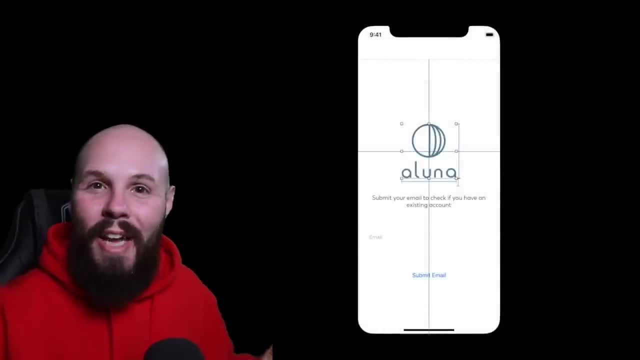 Like: that's a lot of UI code that clutters up your files. So that is one upside of storyboard. Well, depending on how you look at it, it could be an upside is that a lot of that code is on your storyboard right. 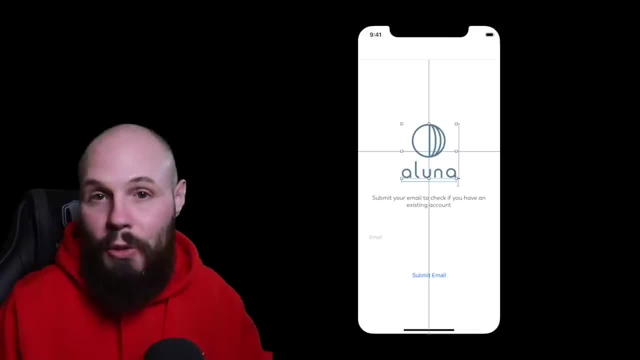 You're not actually coding it, you're setting the constraints there, Whereas when you do everything programmatically, a lot of your code is that UI code. Now the reason why I said- depending on your point of view, if that's good or bad- 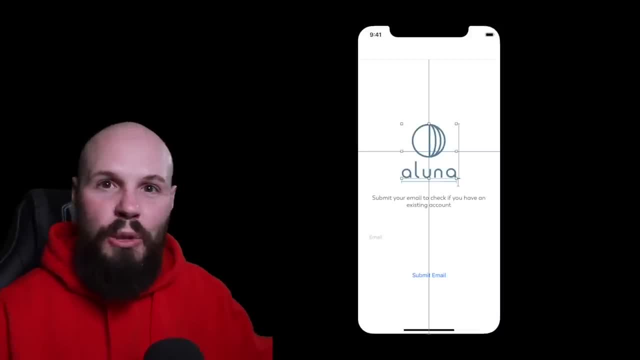 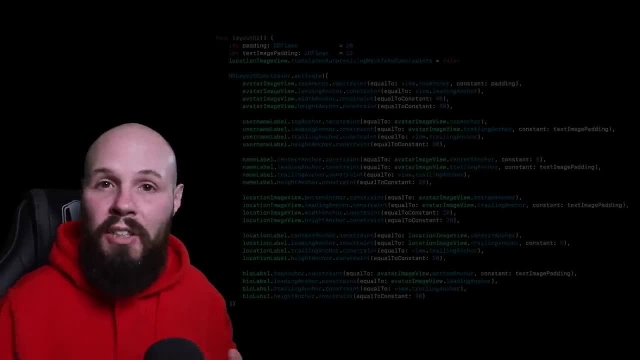 some developers think that when you do all that in storyboard, you're really like hiding it, Like it's hard to decipher what's going on in the storyboard. You have to click into a lot of things, whereas seeing it in code- even though, yes, it is a lot of like cluttered code- 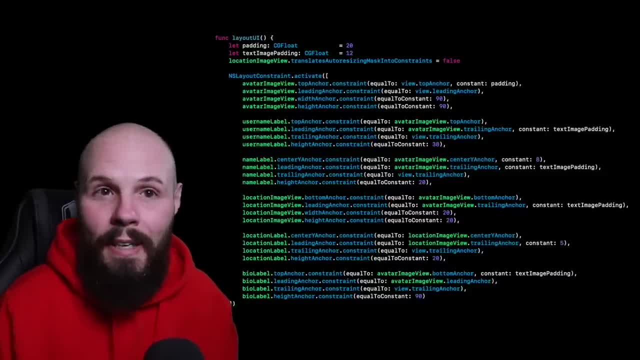 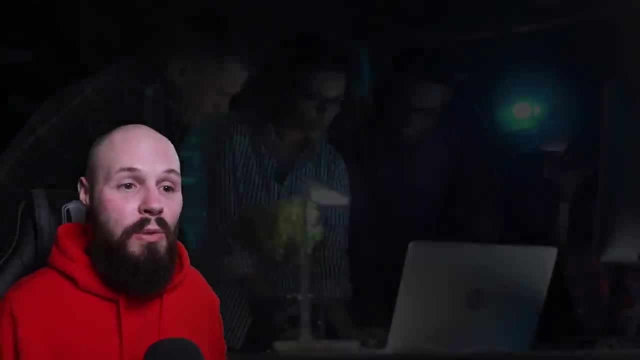 but you can see exactly what's going on right away. It's not hidden. So again you can start to see why there's a debate, right, People have preferences. Another bad thing with storyboards is when you're using them on a team. 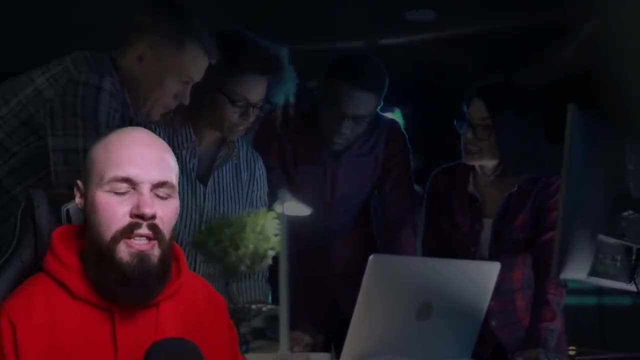 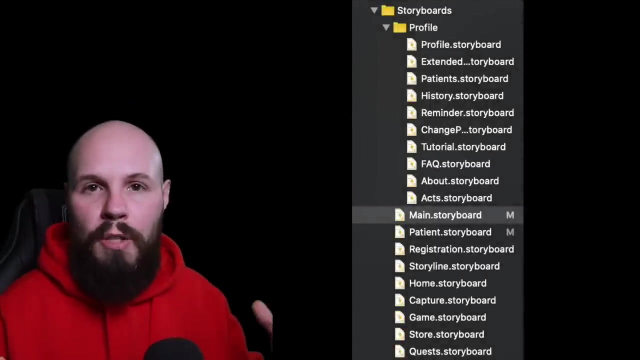 especially a large team like the larger the team, the more difficult it is to work with storyboards. Now remember the Aluna example. I showed you we had multiple storyboards right. So that is a good way to handle this problem, because what happens if you have one giant storyboard? 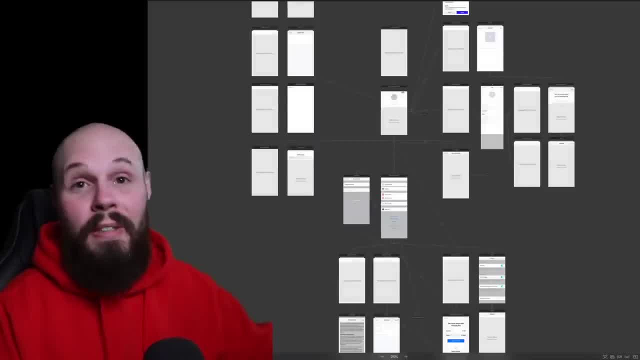 like you saw that nightmare on the screen. well, one thing, that's just a nightmare to deal with, but the way storyboards work. if I'm working on a storyboard and a teammate's working on the same storyboard, we're gonna have a merge conflict. 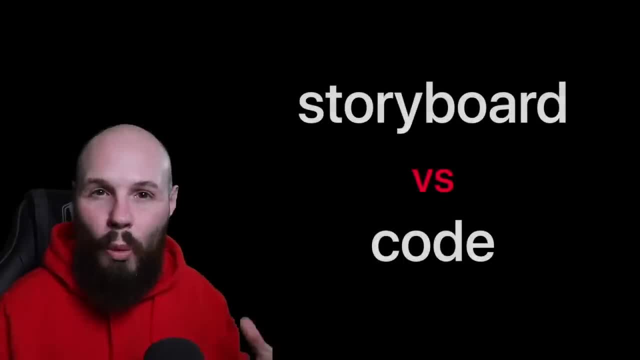 when we go to merge our code and untangling storyboard merge conflicts are a nightmare. Untangling code conflicts aren't that bad. typically You can get some nasty ones, but they're nothing compared to storyboard merge conflicts. So, again, when you're working on the same storyboard, 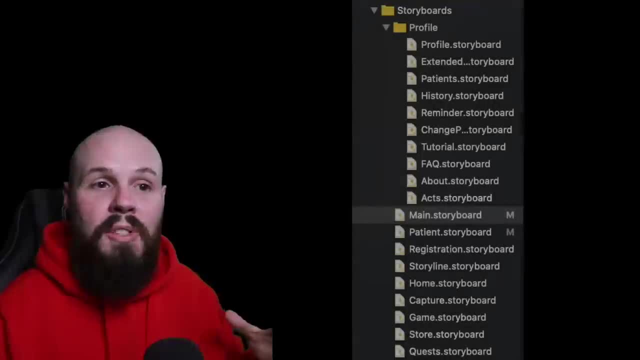 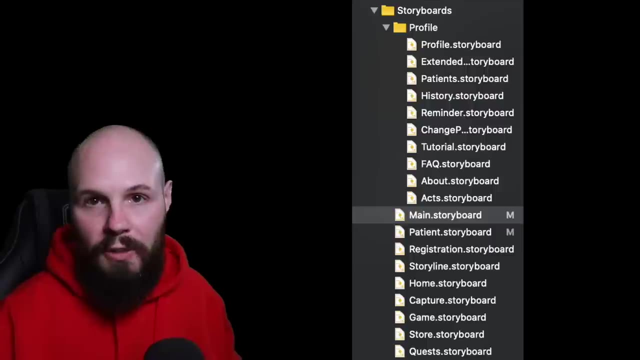 you're gonna get those merge conflicts. That is why it's recommended to separate it out into many, many different storyboards, Because if I'm working on the login storyboard and you're working on the profile storyboard now, we're not gonna have conflicts. 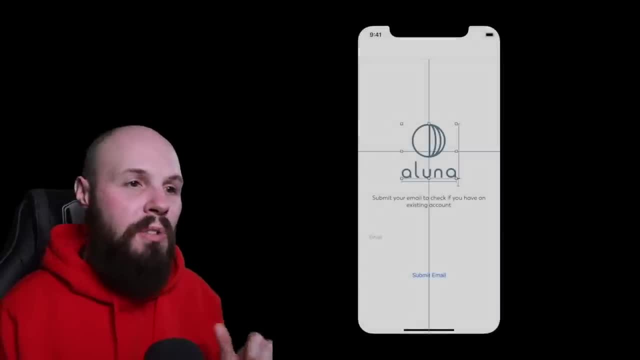 We're in two separate files- no big deal. And another downside of working with storyboards is just the dragging and dropping of elements For super simple screens. it's nice. I really like it. However, a UI gets where you have tons of views. 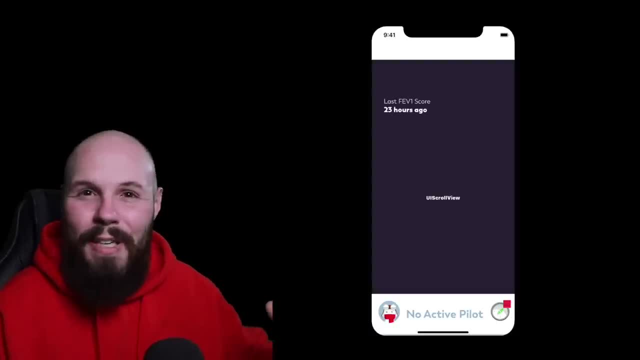 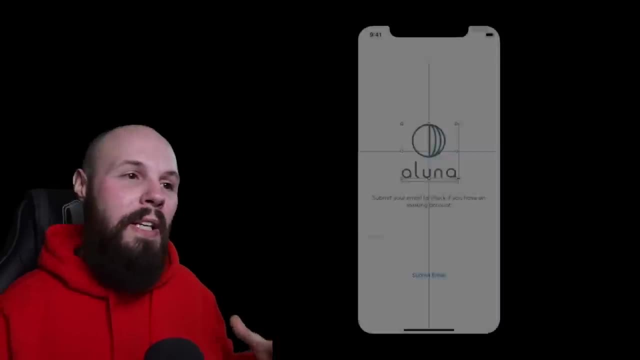 and all the different kinds of stuff on the screen. It's pretty complex, it's dynamic, there's animations. Storyboard becomes a bit brutal to deal with, to be honest with you. So my opinion is like if a screen is super simple, 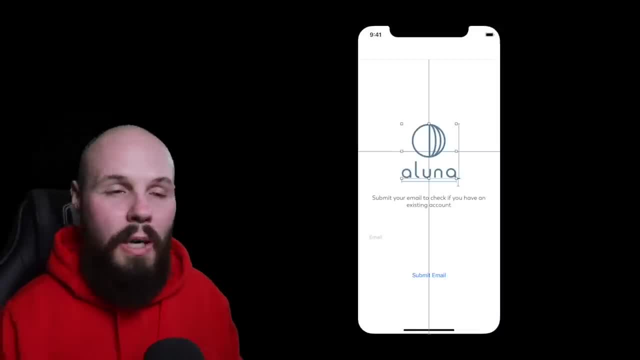 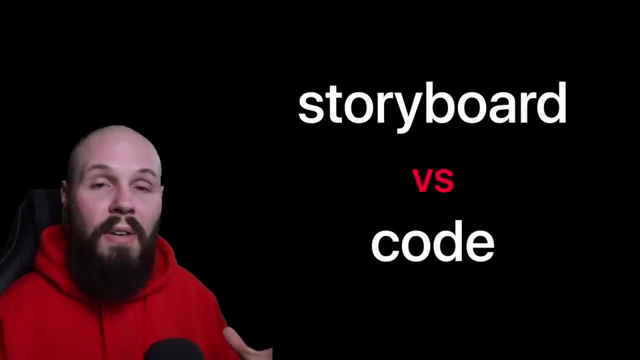 then I tend to prefer storyboard. The more complex it gets, the more I start to prefer to do it in code. So that leads me to some advantages of doing it code. Like I've said before, it's very easy to debug things. 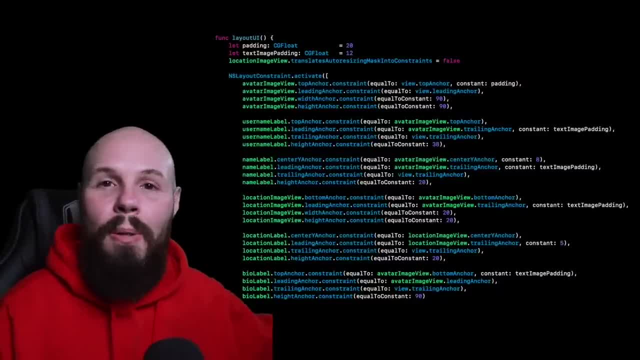 Everything is right there in code. It's not kind of hidden away in the storyboard. It's also easier to build more complex screens because you're not dealing with dragging and dropping elements on the storyboard. It's also easier to make changes right. 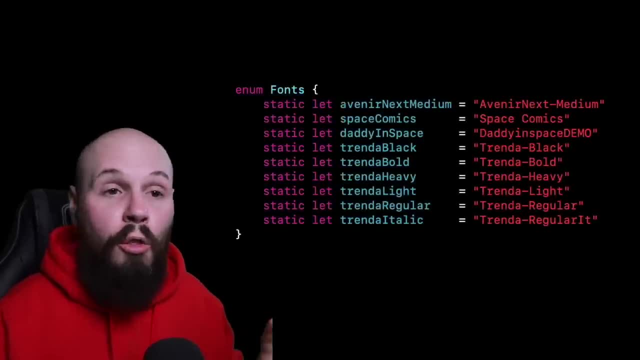 So if I wanted to change the color of a button or the font all throughout my app in storyboard I would have to go to like each individual element and like: change the font of this label, change the font of that label. Like it's annoying to go through and change all the elements. 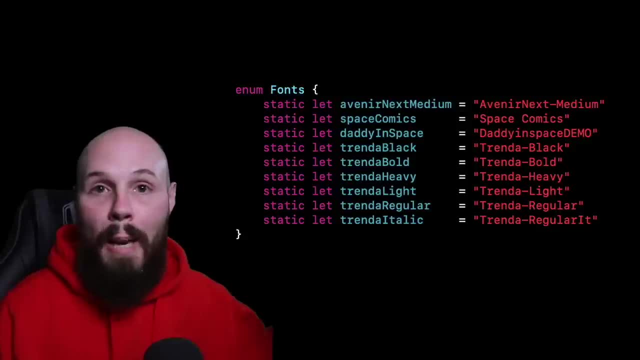 Whereas if you do things programmatically and you can set, like a, here's my app font as a constant and you use that app font through all the elements, all your code, now you just have to go to your constants file, change that one font. 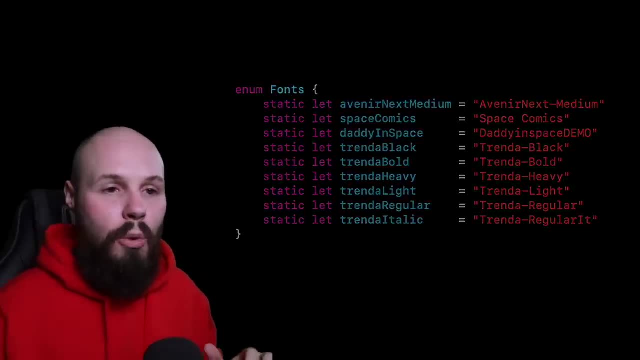 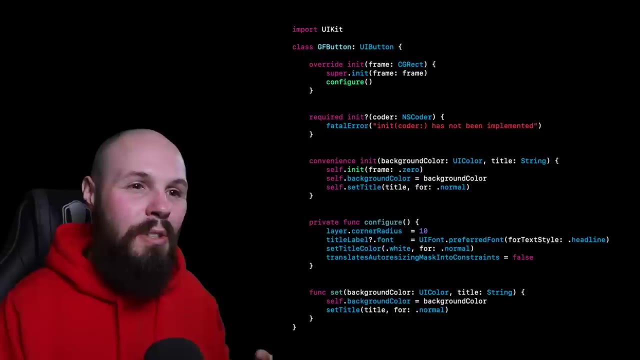 and it's changed all throughout your code. So building everything in code allows for a lot of flexibility. It's also good for reusability, right. It's very tricky sometimes to copying and paste stuff from the storyboard onto another storyboard or a certain UI element. 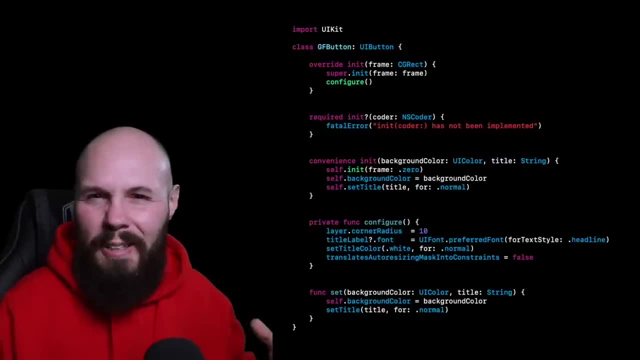 It's possible for sure. It just can be tricky and a headache, Whereas copying and pasting just a chunk of code and maybe making some small changes, that is super fast and easy. So, like I said, building things in code, while it may be a little bit more work, upfront right. 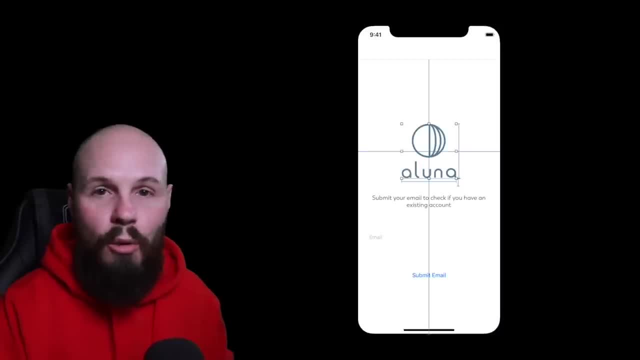 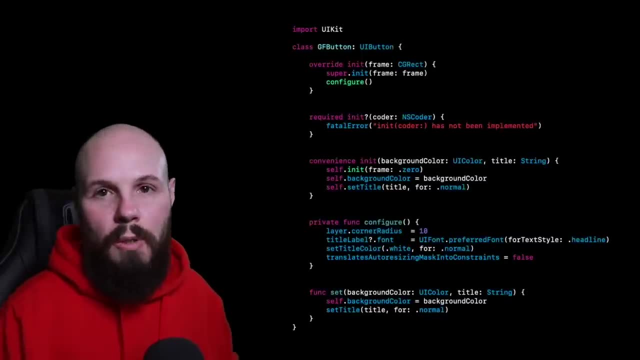 It's a lot easier to drag an item onto the view controller- constrain real quick done- than to like type everything out in code. But again, you're gonna get a lot of flexibility when you build it in code. So again, how I feel about it, it's on a spectrum. 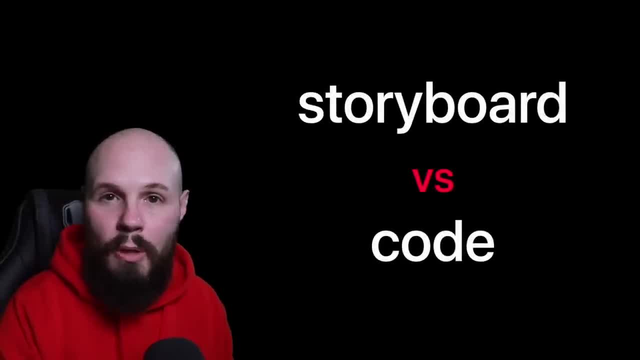 The easier the screen on that spectrum, the more I prefer to do in storyboard. If it's just super simple, maybe two or three elements on the screen, straightforward, I prefer storyboard. Again, as it gets more and more complex, the more I lean towards you know. 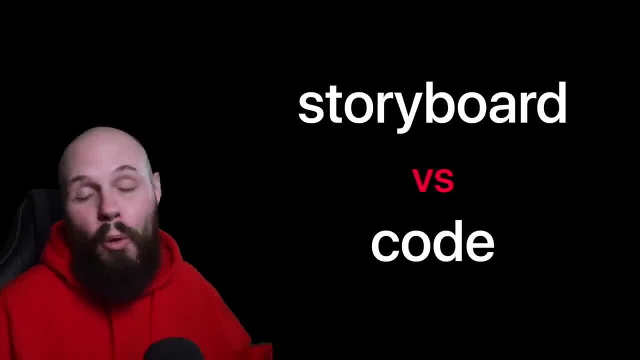 doing it in code. That's just my opinion. You're gonna form your own over time as you build projects in both. but that's a good point. At the end of the day, it's perfectly fine to have a preference. Like I prefer code, I prefer storyboard. 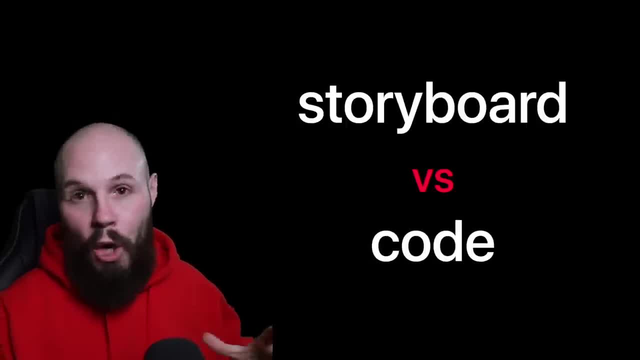 Fine, have your preference, Although a lot of people on the internet are gonna tell you you're wrong. no matter what preference you choose, that's the internet, But I do think it's very valuable for a developer to know how to do both. 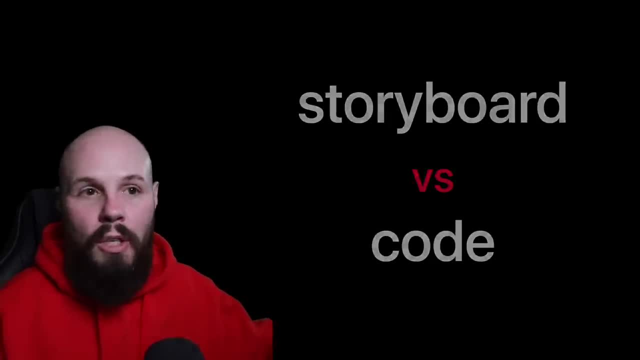 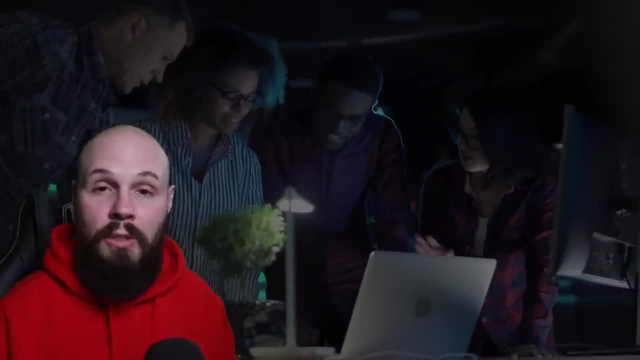 And here's why is because, even if you hate using storyboards, you should still know how to do it, Because if you get a job, you get a contract, you join a team, whatever that is, and that project's built in storyboards. 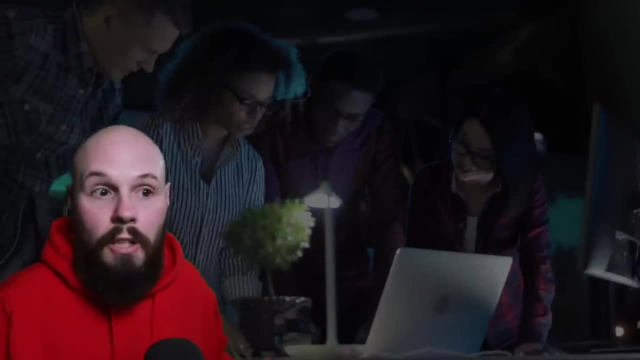 like you're not just gonna be able to stomp your feet and say I'm doing it in code, Like you're gonna have to fall in line and start using storyboard. So that's why I think it's super important to know how to do both. 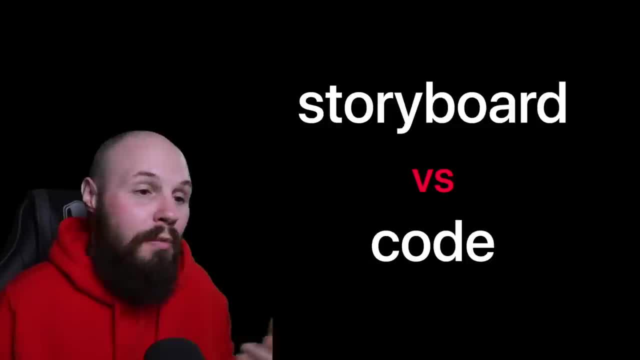 It's gonna benefit you greatly to be flexible as a developer Like I'm. perfectly comfortable with both. You throw me in a storyboard project- I'm good to go. You throw me in a 100% programmatic project- I'm good to go. 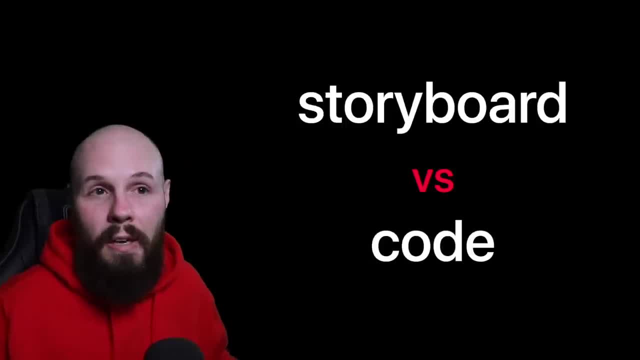 You throw me in a project that's like a mix of both. I'm good to go And I think that's what you should strive for. That's just my take on it. Like I said, it's a hotly debated topic. 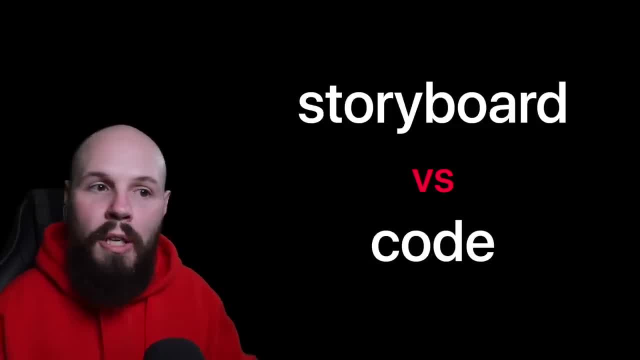 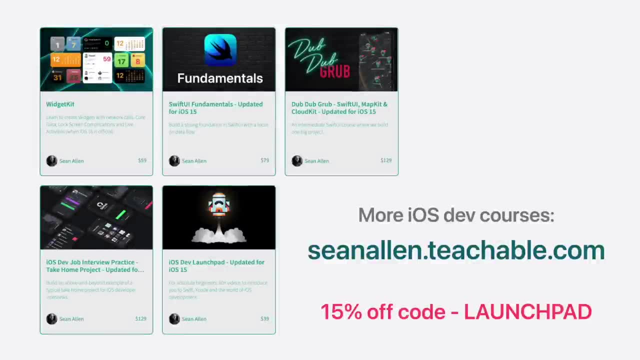 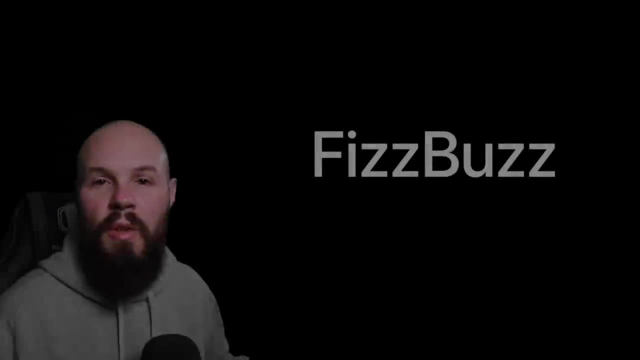 but I'm hoping in this course I can show you a little bit of both and you can start to form your own opinions based on experience, not what someone tells you. So all right onto the next video, Now that we've learned the basics of the Swift language. 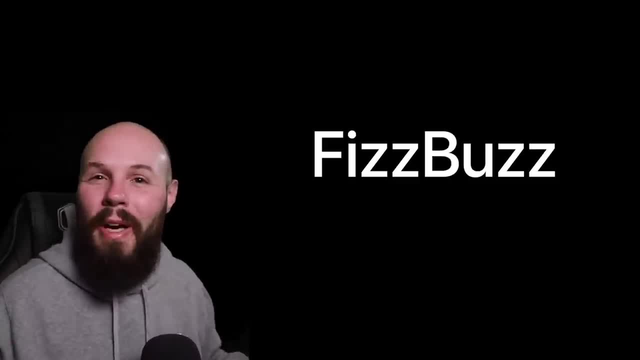 let's talk about fizzbuzz. Fizzbuzz is kind of like a rite of passage for beginner programmers. It's a short coding process that you have to go through a lot of times And it's a problem that oftentimes you'll do. 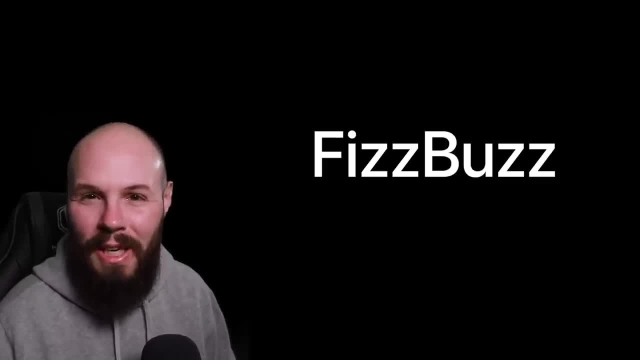 when you're just learning a language. So if you ever decide to pick up another language, you'll probably do fizzbuzz in that language as well. But anyway, I'm going to explain the requirements of the problem to you. However, I encourage you to pause the video. 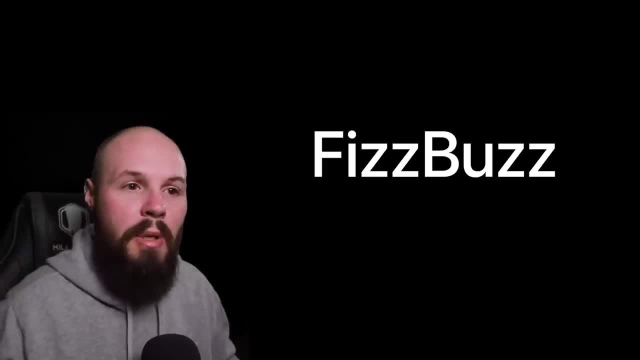 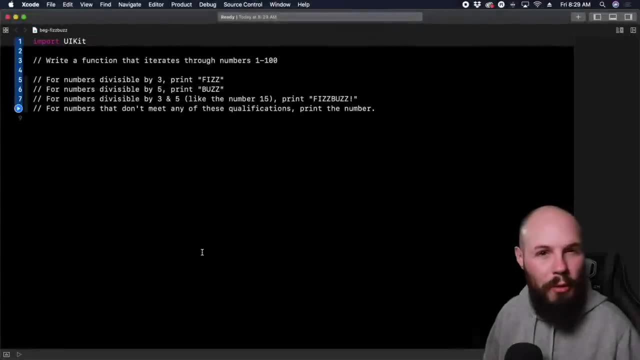 Like: of course we're gonna walk through the solution and I'm gonna explain everything, but pause the video after I give you the instructions and try to solve it yourself. Here I am in a new playground. Hopefully you can create those by yourself by now. 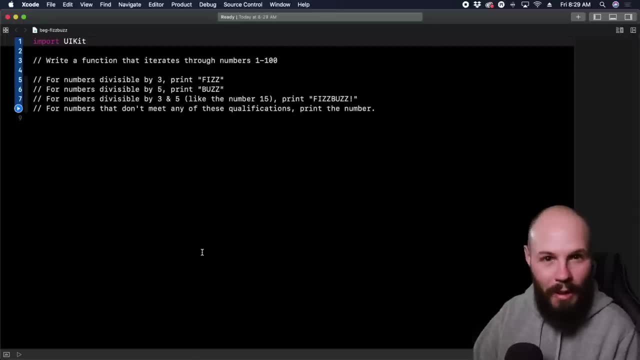 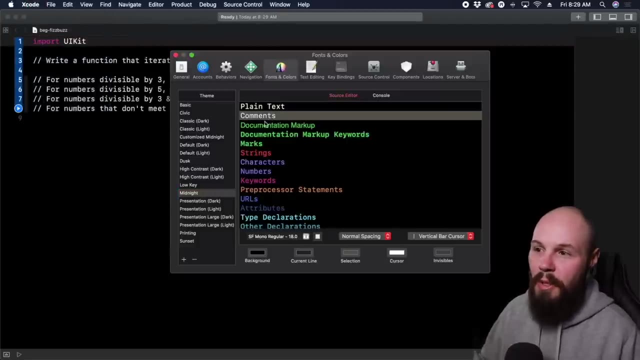 And you can see the instructions here. a little side note in case you're wondering why my comments look different. I changed the color to white Again. if you remember Xcode preferences, fonts and colors, you can change your comments. I just changed those to white. 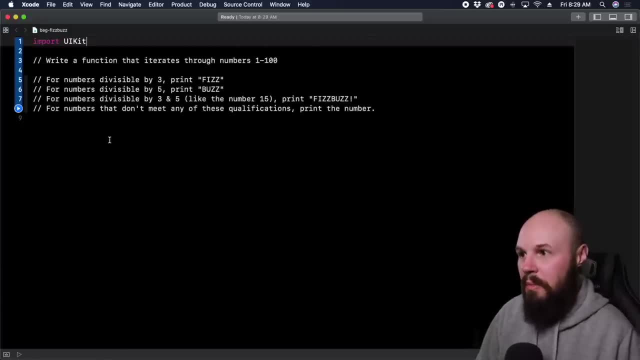 in case you're wondering how that happened. Okay, so here are the instructions. Write a function that iterates through numbers one through 100.. And as you're going through that list of numbers, one through 100,, if the number is divisible by three, print fizz. 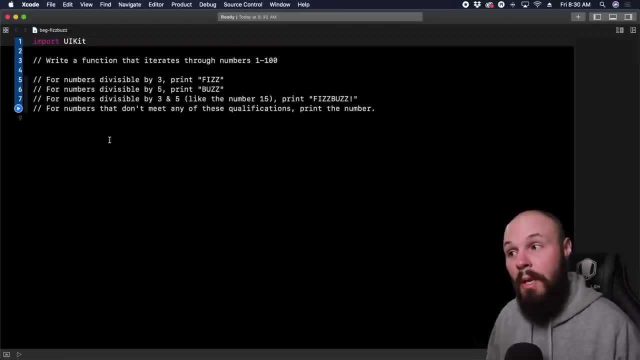 If the number is divisible by five, print buzz. If the number is divisible by three and five, like the number 15, that's when you print fizz buzz with the exclamation point, And then if the number doesn't meet any of those requirements, 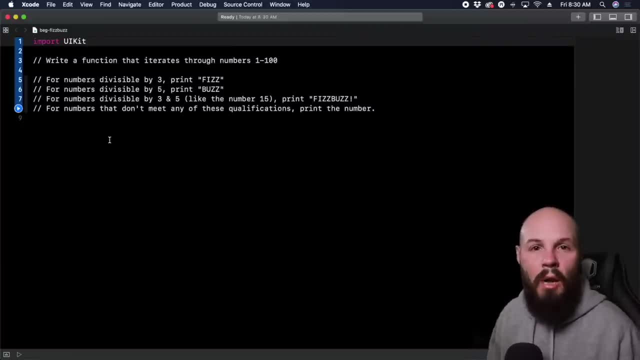 go and just print out that number Now, when I'm solving problems like this, oftentimes I'll break out a pen and paper, or maybe my iPad and my Apple pencil actually get some use out of it, But don't worry about coding this right away. 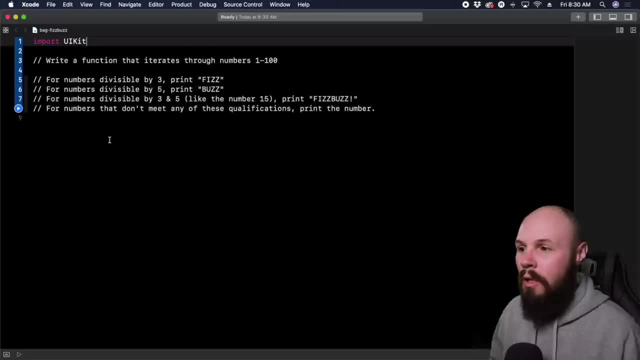 when you're trying to solve these problems, Like again, if you're gonna take this on on your own, bust out a pen and paper and start kind of scribbling down- like some we call it pseudo code- on what you would do. 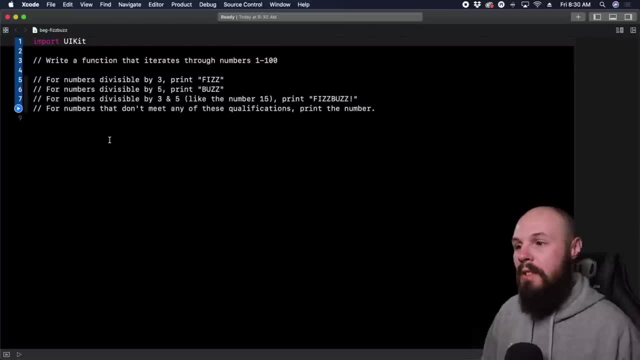 For example, you know like if the number is divisible by three, do this right. So another hint is that everything you need to solve this problem we've already covered in previous videos. So if you find that you're solving this problem, 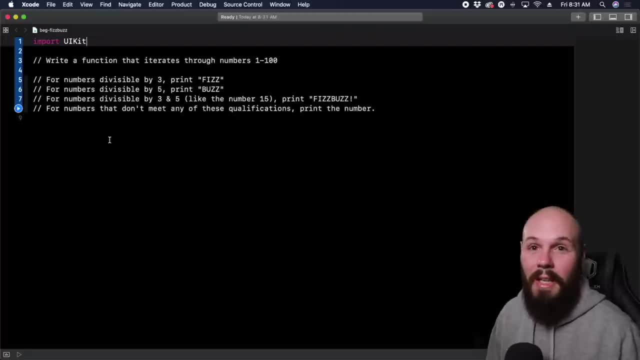 with stuff we haven't talked about. you're probably doing it wrong. All right, last chance to pause. Don't look it up either. We're gonna solve it right here, Don't Google it. So, anyway, last chance, pause right now. 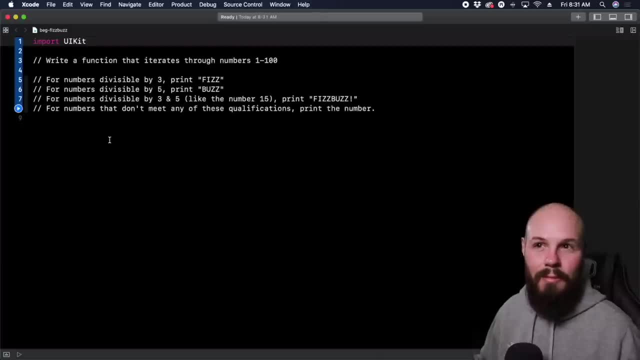 After two seconds, I'm going to continue One, two. all right, let's go. So let's talk through this first And again. this is how I would try to tackle these problems, again with pen and paper in hand to take notes. 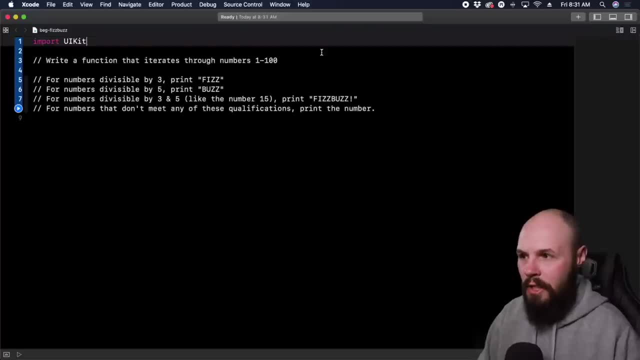 So, okay, looking, we need to write a function. Okay, so we're writing a function that iterates through numbers, one through 100.. Okay, I see, iterates through numbers. I'm thinking of for loop, right with a range. 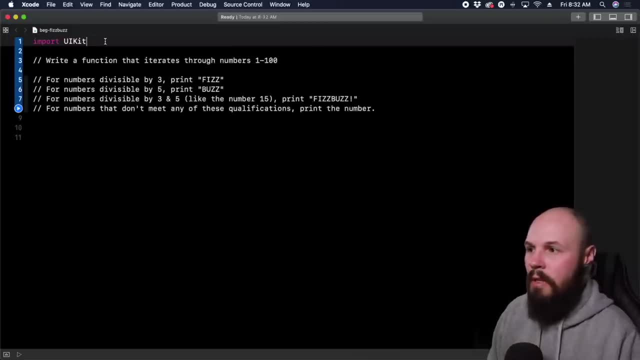 Okay. so I'm gonna write a function with a for loop, one through 100, to iterate through that, Okay. and then for numbers divisible by three, print fizz, Okay. so if that number is divisible by three, I have to print fizz. 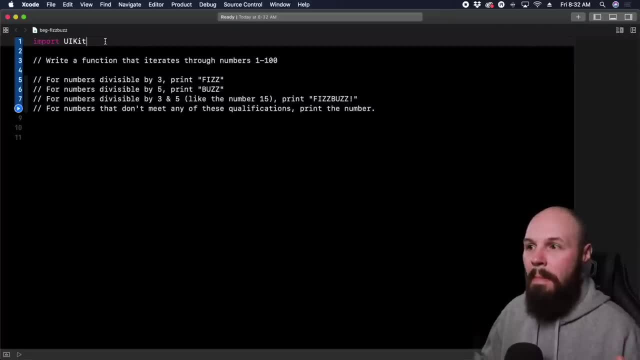 Okay, so I know how to do an if statement. I'm gonna print out fizz. How do I know if the number is divisible by three? Well, do you remember the modulo operator? Well, remember that returns just the remainder. Well, if something is divisible by a number, 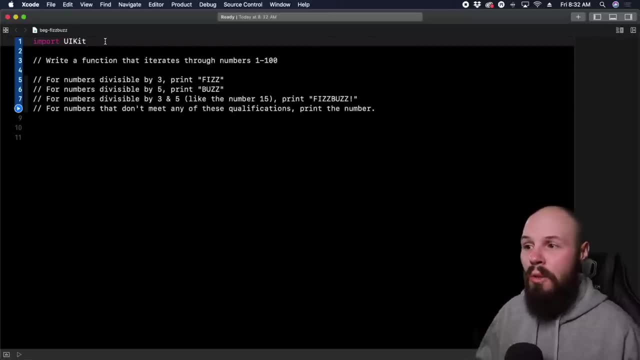 the remainder is going to be zero, correct? So if you use a modulo operator on the number and the remainder is zero, well, you know it's divisible by three, Cool. so that's how you handle. the is divisible by. So I guess the same thing applies for five, right? 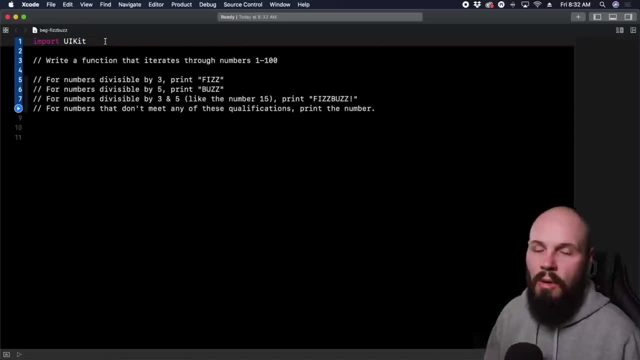 You know, use the modulo operator on five If that number equals zero. you know, print fizz. But now we run into this case here on the third line for numbers divisible by three and five. Okay, because right, if we check for a number that's divisible by three, 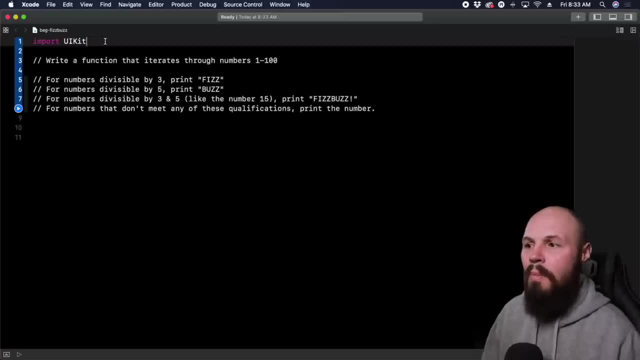 and then just move on. well, what if it was divisible by five as well? So here we can use the and operator to check, Like, if you know, using the modulo operator on three equals zero and you know, modulo five equals zero. 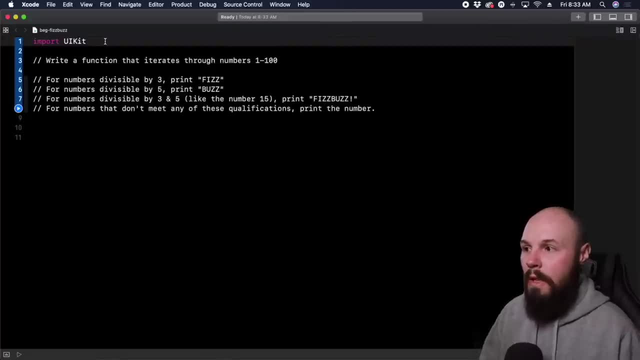 Cool, now we know it's divisible by both. Okay, And then, of course, if the number doesn't meet any of those qualifications, we're just going to print the number. Okay, so it looks like we're using if statements, modulo operators for loops in a function. 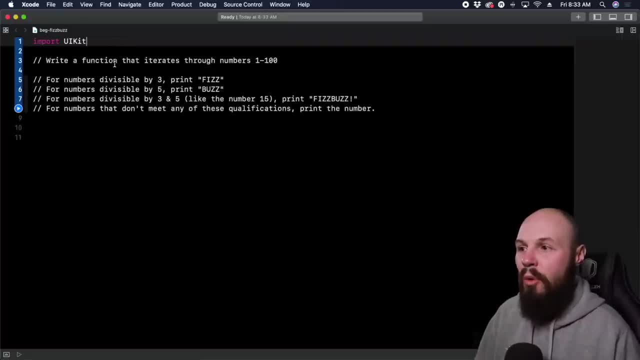 but the order matters, Remember, like I just said, like we can't just check for if it's divisible by three and move on. So we should probably check first if it's divisible by three and five And then if that's not true. 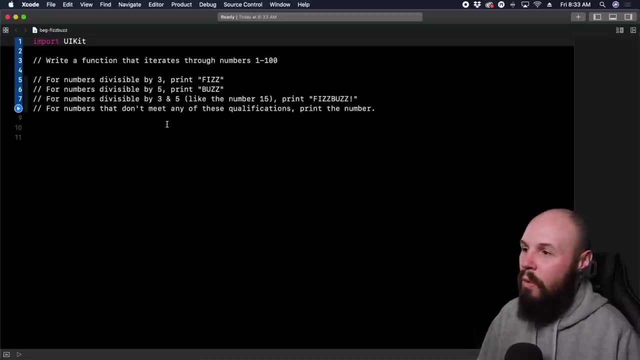 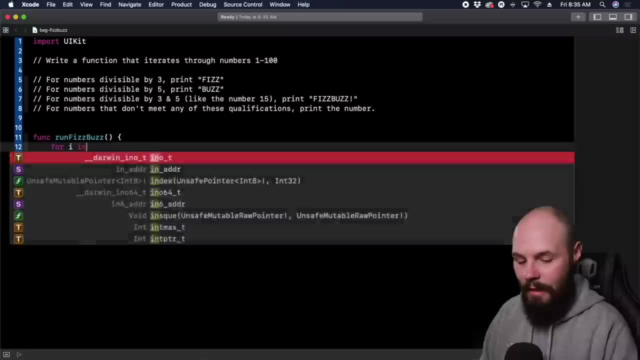 then move on to three, then move on to five. So that's kind of the order that we're going to do it in. So let's actually start writing this Func, fun, fizz buzz for i in one dot, dot, dot 100. 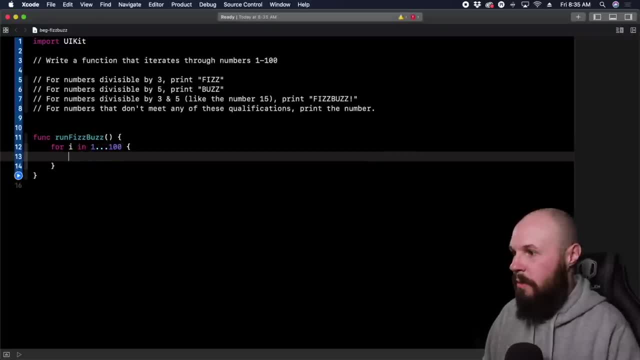 So that's going to go one up through 100.. So we're going to get all those. Okay, there's my for loop, All right. So now we have our for loop and it's telling me: I haven't used, i yet. 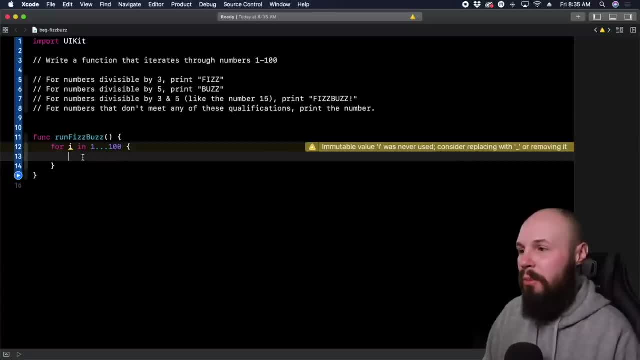 We're going to use. i Remember our first check is going to be if it's divisible by three and five. So let's do that. So if i modulo three equals equals zero. So this is us seeing if the number divided by three has a remainder of zero. 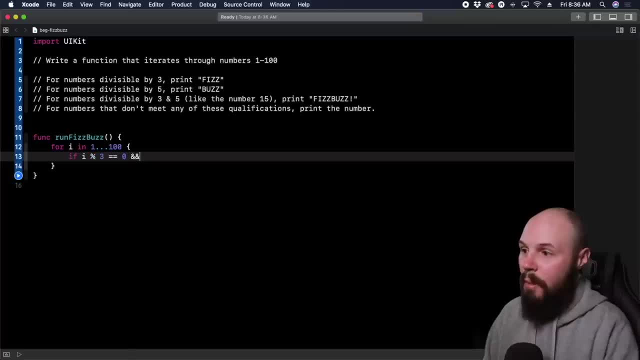 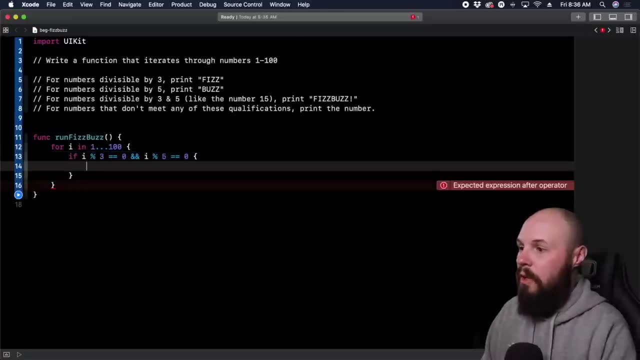 That's what we're saying here, And we want to use the and operator. So, and remember we went over that- i modulo five equals equals zero, So here is this case handled. So now we want to print. This is where we print fizz, buzz. 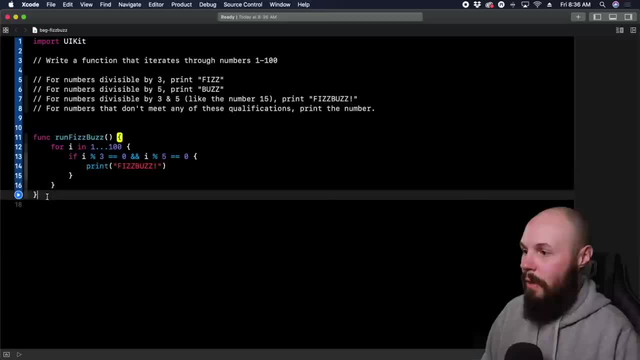 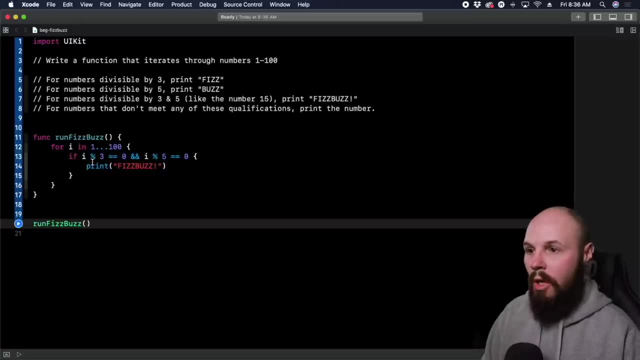 We got it, So let's actually test this. So down here, we actually remember: call your functions, So run, fizz, buzz. So now let's see if this is working so far, And this is another thing you want to do- Is you want to test your code along the way? 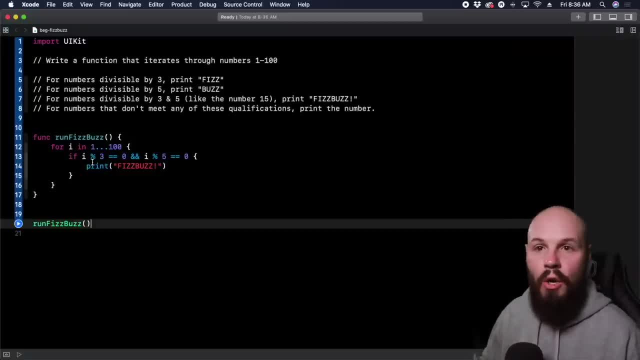 because if you just spend an hour writing out all this code and then you test it, it's a lot harder to debug if something goes wrong, because you have all this code like ah, what went wrong? Whereas if you kind of test it along the way, 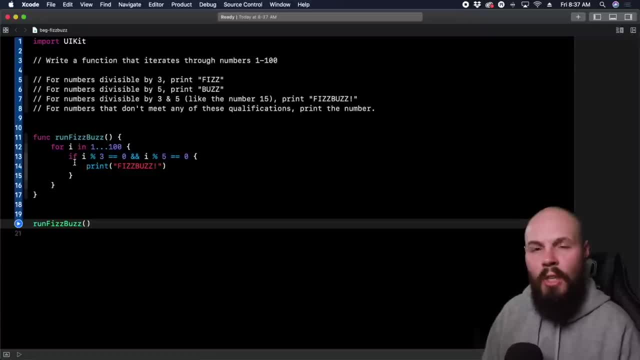 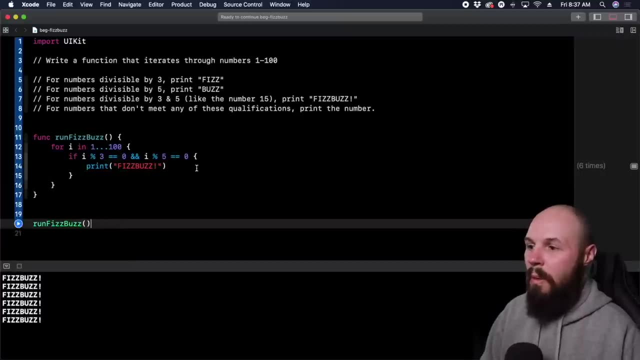 like right now. we only have this small piece of code, So it's very easy to know where the problem is, if there is a problem. So let's run this and it does print fizz, buzz six times, but we don't know what the number is. 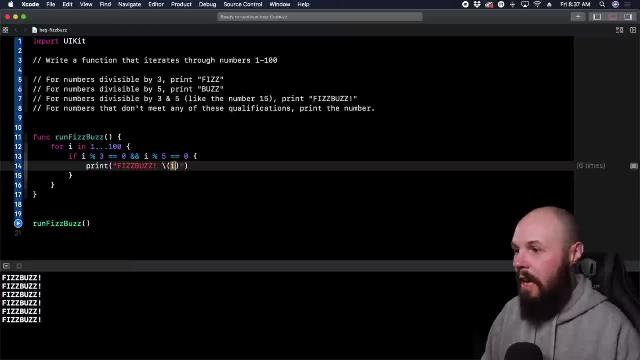 So let's actually add something here temporarily. So again, string interpolation. i We'll print the number after fizz buzz. So run it just to check. So 15, 30,, 45,, 60,, 75,, 90.. 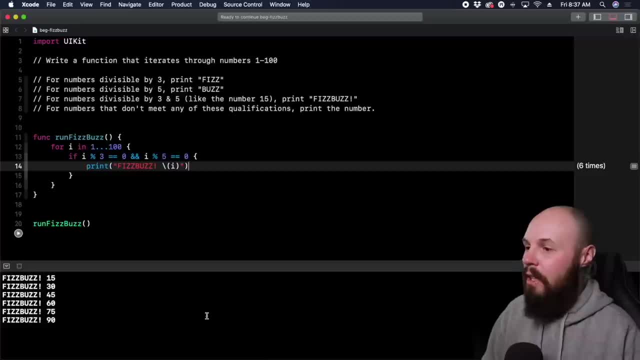 Yep, those are the ones that are divisible by both three and five. And again, I just wrote that to check So we know that's working so far. We can delete that. So now we can stop this with this little. stop button down there. 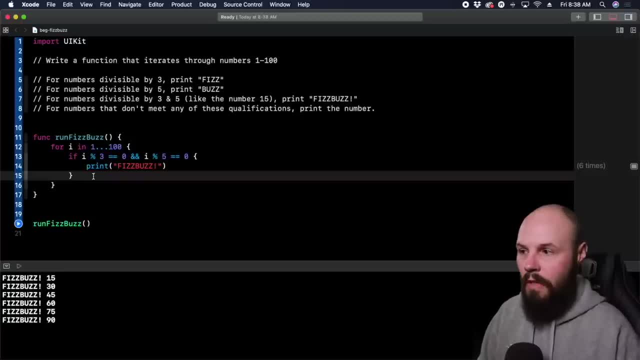 Okay, so that's the first check. So the next two checks are very, very similar, right Else, if I modulo, three equals equals zero. So this is the circumstance where we're checking if it's just divisible by three. 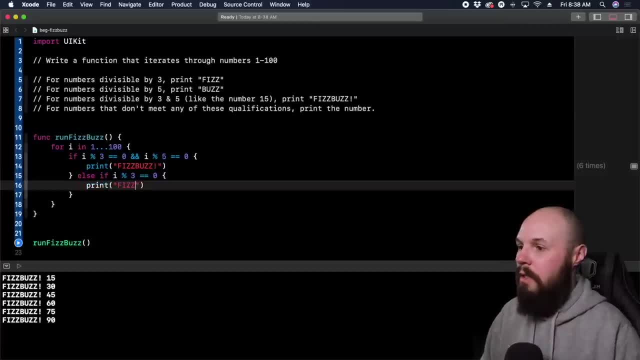 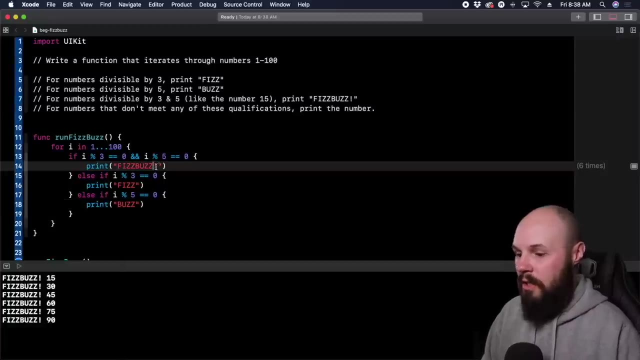 So this is where we want to print fizz And now we do else. if I modulo five equals equals zero, print buzz And you know what? Let's actually keep that in here, just to check right. So again, string interpolation I. 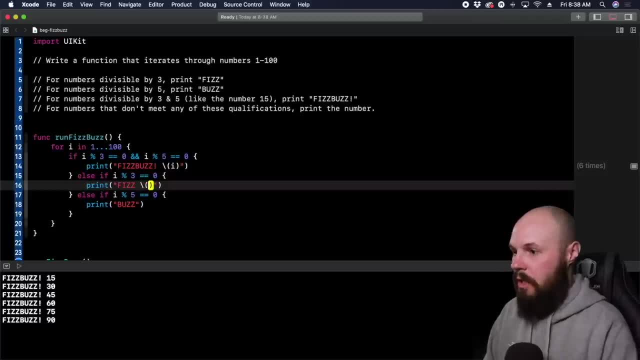 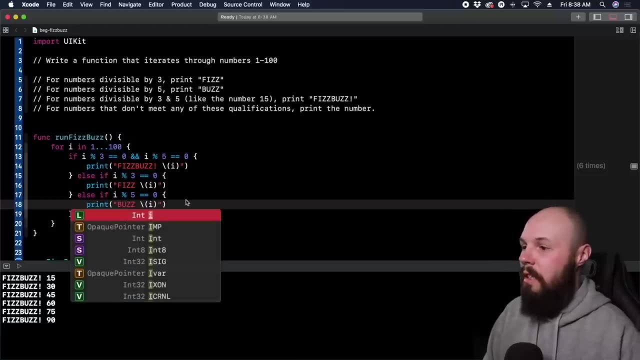 oops, string interpolation I, because this will print the number after it, And then again string interpolation I, just to check. I know that's not part of the instructions, but this will show you that it's actually working like we showed before. 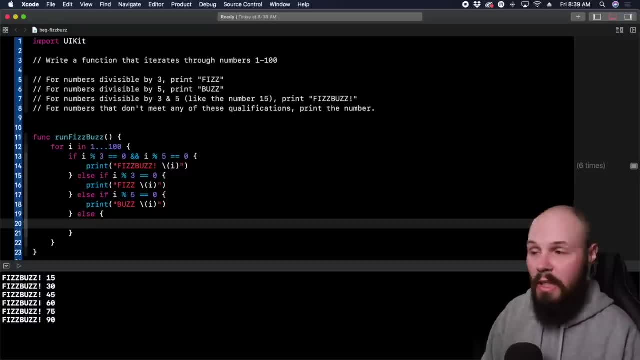 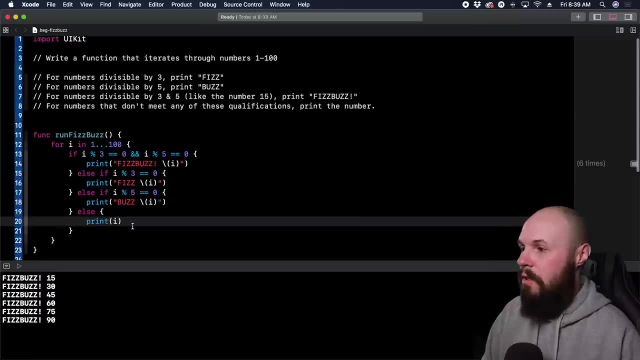 And then else right, If it doesn't meet any of the requirements, being divisible by both three and five, divisible by three, divisible by five, we want to print just I. So there's our quick function. Again, let's run through it just to really reiterate. 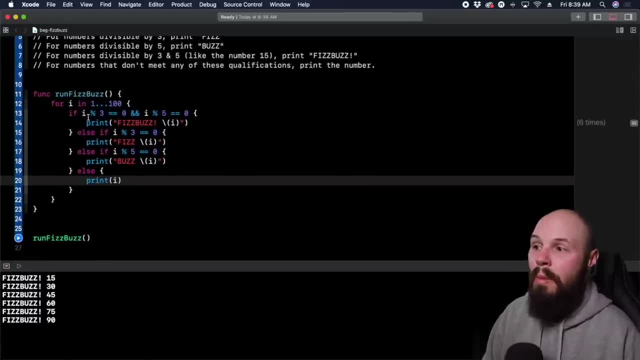 We do a for loop going numbers one through 100.. If it's divisible by both three and five- that's what we check first- We're going into this. we're printing fizz buzz. If it's divisible by just three, we're printing fizz. 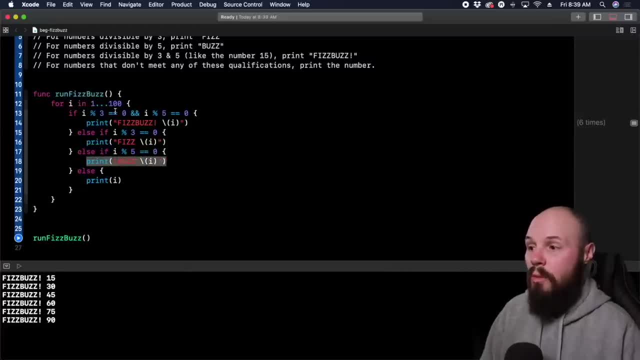 If it's divisible by just five, we're printing buzz. If none of that triggers, we're just going to print the number. So now let's run fizz buzz here and we'll make this real big so you can see it right. 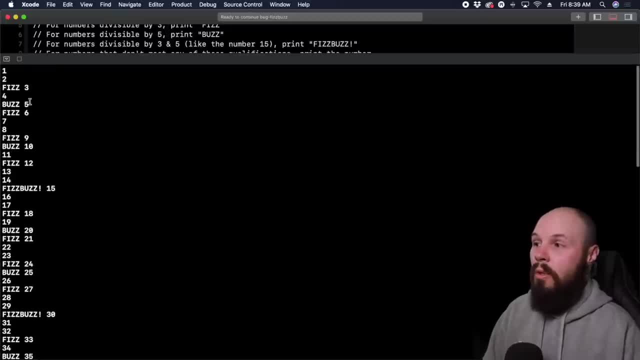 Scroll up to the top right: One, two, fizz for three, four buzz for five, fizz for six. right, And I'm not going to go down to the whole line, but you can see our fizz buzz is working. 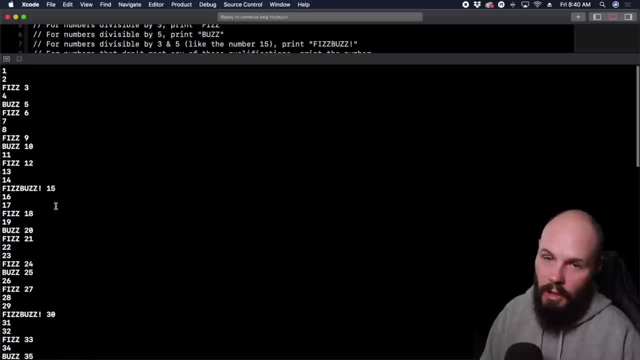 And then we get our first fizz buzz at 15, which again makes sense. So, and you can see, we go all the way through 100, doing fizz and buzz if it's divisible by three or five respectively, and then both. 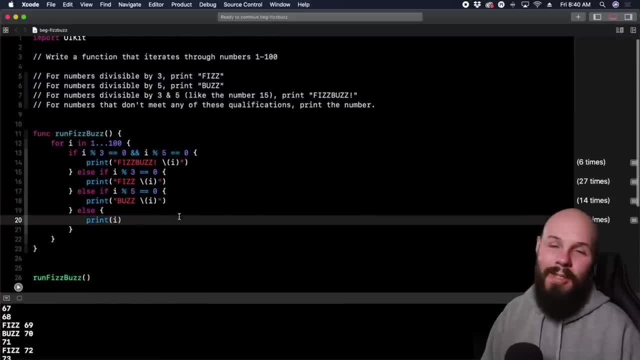 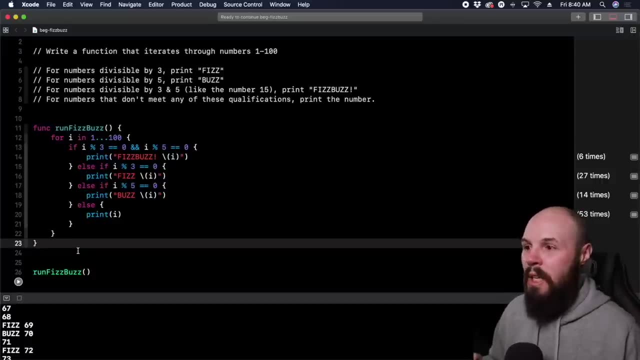 So again, fizz buzz is a classic right of passage. You're probably going to see this a lot throughout your programming career. when you're just learning other languages should you decide to explore those. But, as always, if you have questions on how we came up with the solution or concerns, 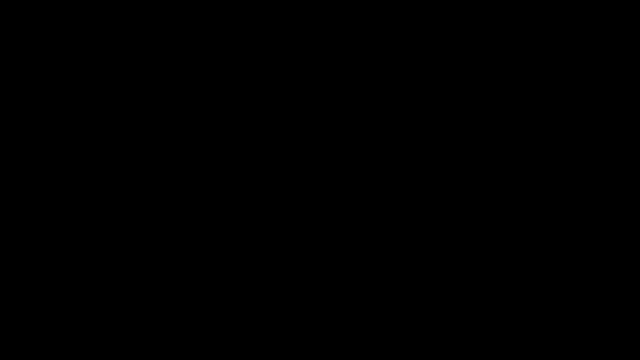 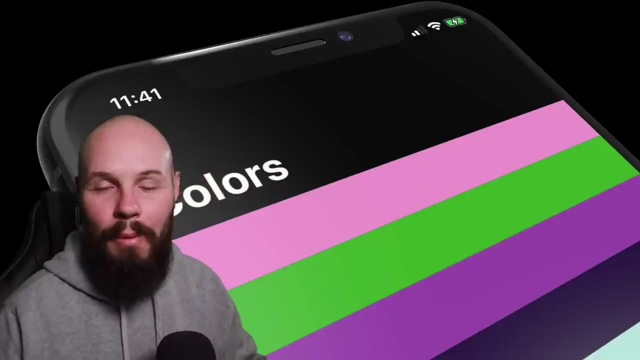 leave a comment or hit up the Slack channel and we'll see you in the next video. All right, we're about to build our very first beginner app. We're going to keep it simple, don't worry, But in this video I'm going to show the overview. 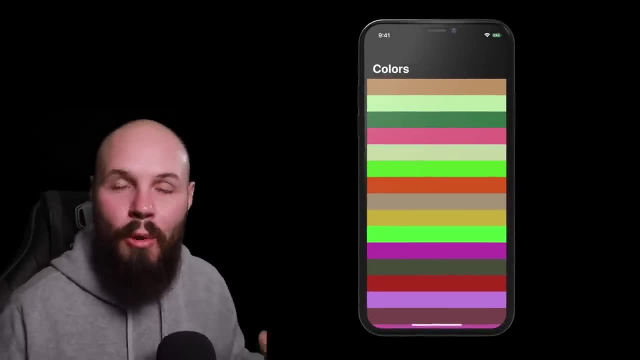 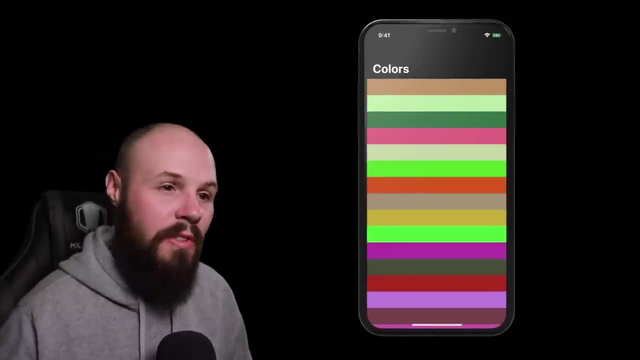 of what the app is going to be and some of the topics we're going to learn throughout the next couple of videos. The functionality is actually very simple. As you see on the screen, we're going to have a table view that populates with 50 random colors. 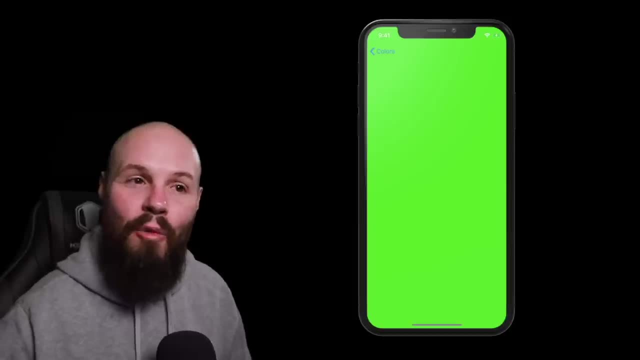 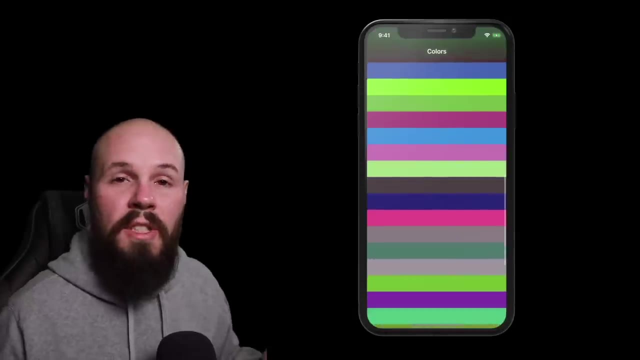 And then, when you tap on one of the cells, we're going to pass the data of what that color is to the next screen and change the background color of that screen to the color we selected. Looks super simple, right, But we're actually covering a decent number of topics. 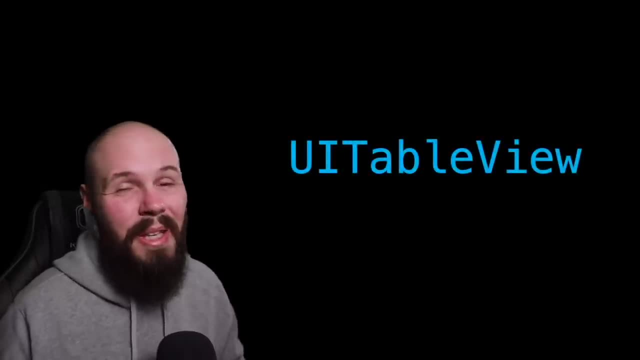 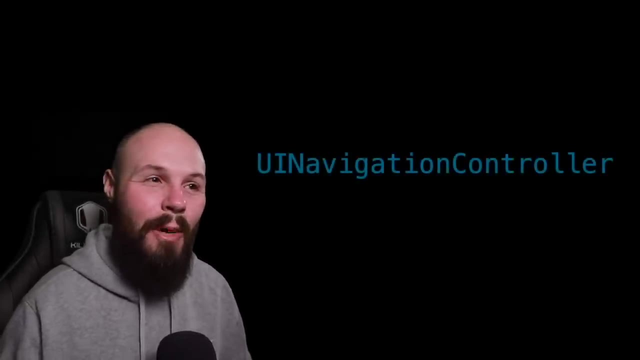 in this app, For example, we're talking about UI table views. That's a big thing for developers, right? There's table views all throughout apps. That's probably the most common thing you're going to build. We're also talking about UI navigation controllers. 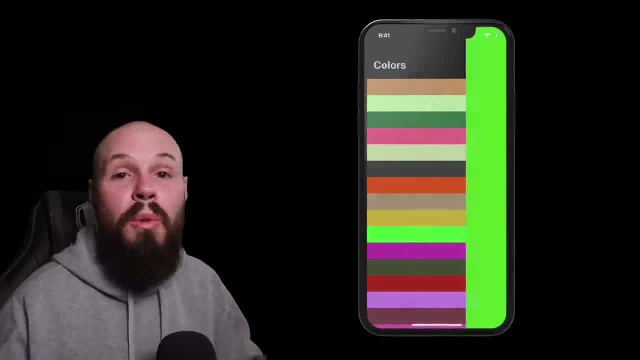 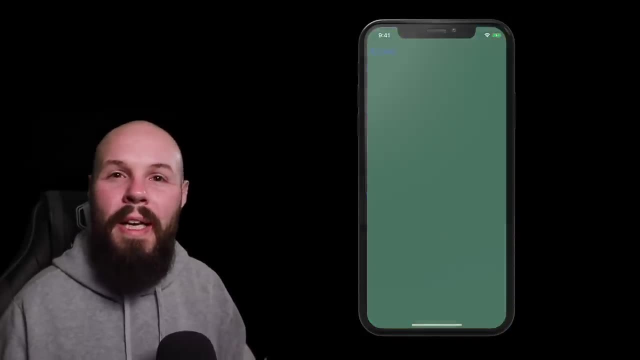 for loops, arrays, passing data from one view controller to another- like that's another big skill- And then also generating random numbers, which we've kind of touched on already, And we're going to create an extension on UI color that will spit out a random color for us. 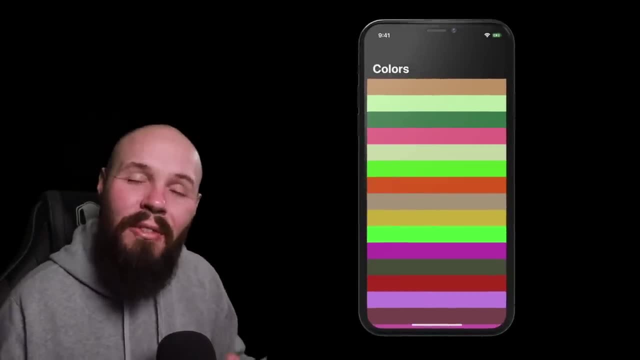 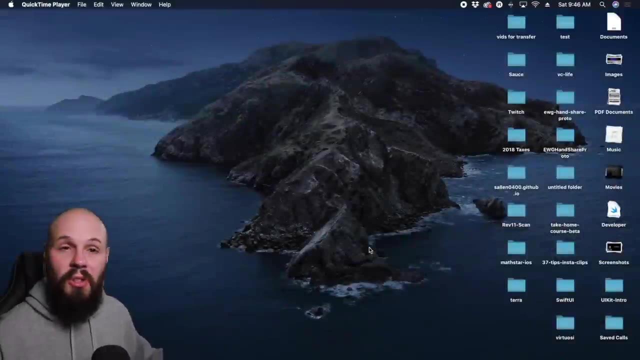 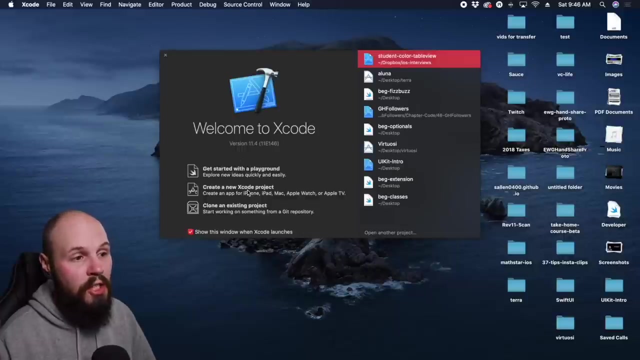 So, again, the functionality looks pretty simple, but we're actually covering a lot of topics. All right, let's get right to it. Of course, to start this app, we got to open up a new Xcode project. So pull up Xcode. create new Xcode project. 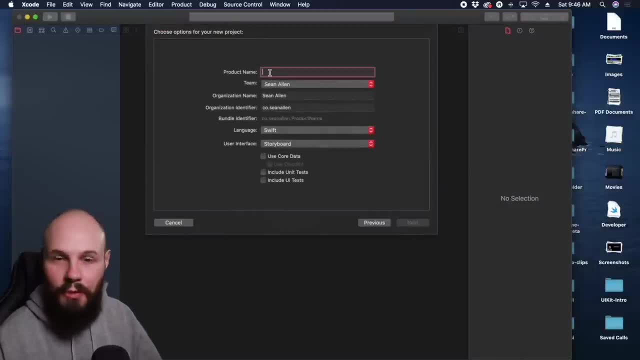 single view application next. Hopefully you've done this before by now. Product name- we're going to call this random colors And again, team is whatever your team is, organization name, et cetera. Swift and storyboard hit next. 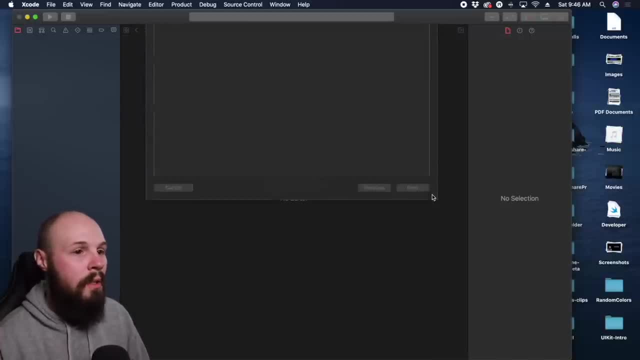 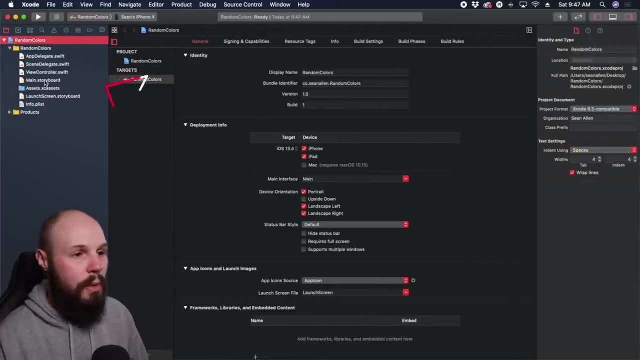 And save it to. I'm going to save it to my desktop, You can save it to wherever you like, And we're going to make my Xcode fill up the whole screen here. Okay, cool, Click on your mainstoryboard. 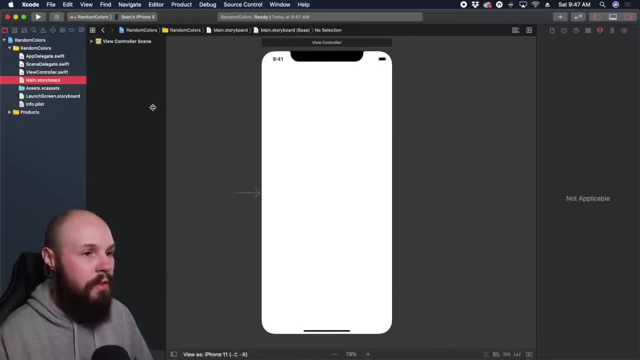 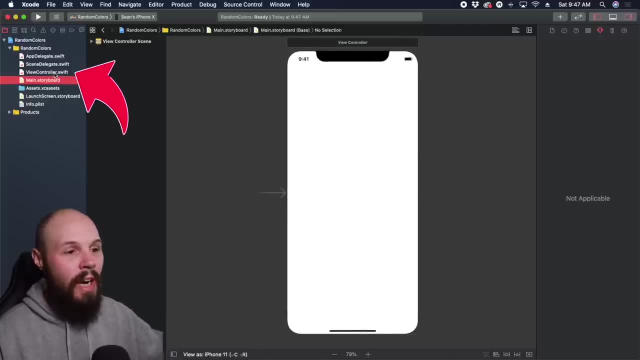 And what I'm going to do here, as I just make room here for my giant resolution screen- the things I do for you. So you see, we get a view controller from the start. We get a view controller file. It's our initial entry point here. 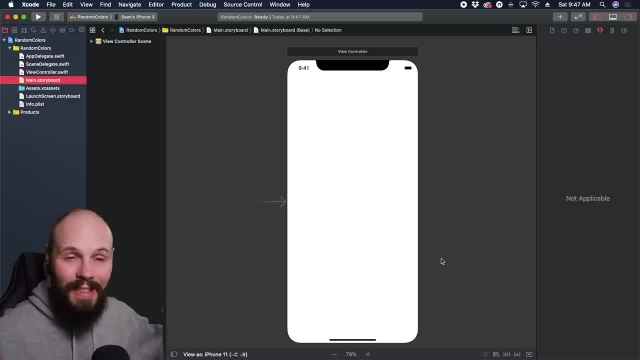 as you can see in this arrow. So they do give you a basic setup. I'm actually going to tear all this down and build it back up from scratch, because I think that is better for you to understand how this all comes together. So if you click on this storyboard, that bar up there. 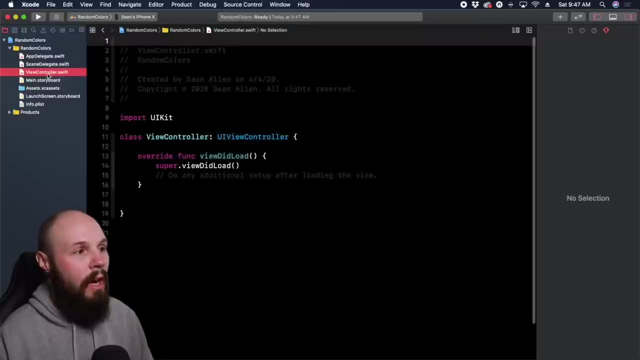 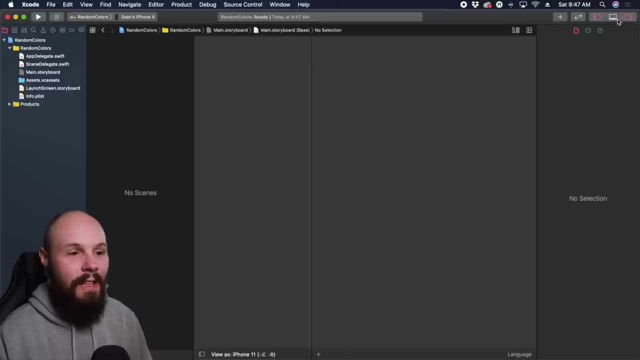 just hit delete. that'll get rid of that. Click on the viewcontrollerswift file. right click delete. move to trash. That is gone. cool, Now you can see this empty storyboard here, So what I want to do is hit the plus button. 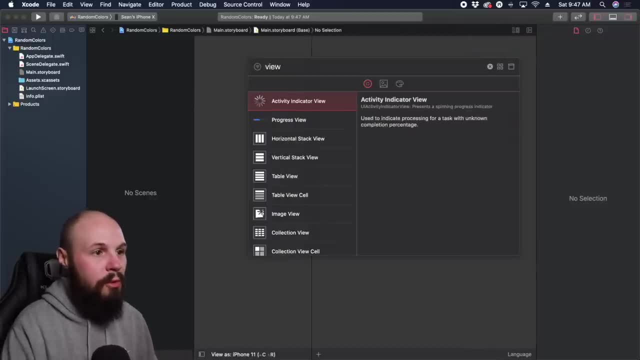 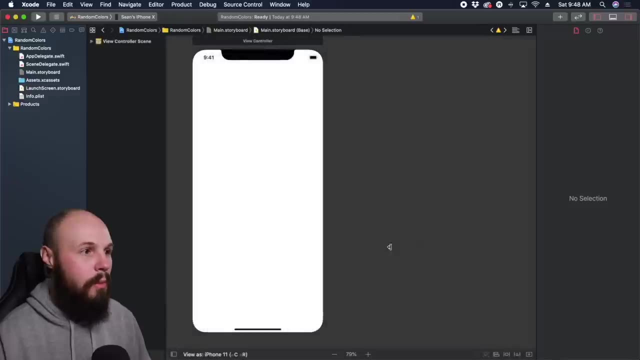 go. or you can do command shift L if you remember, but you can hit the plus button view controller. There we go. Okay, let's all. my sizing of my screens are all messed up. You go away. Whoa, yeah, okay. 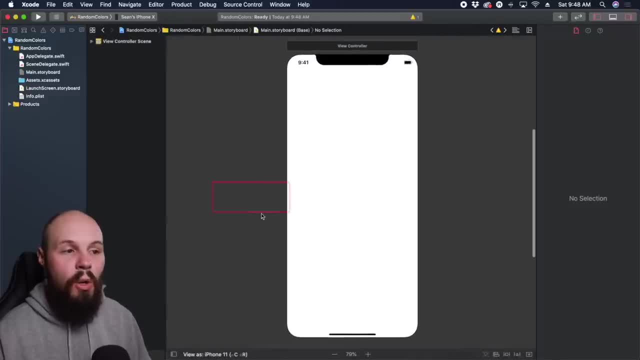 There we go. So here's my one view controller on the screen. You see I no longer have that initial entry. We'll come back to that in a second, But the way the storyboard works is all the view controllers on the screen. 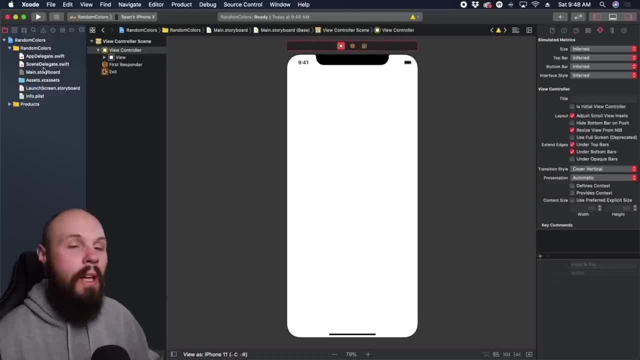 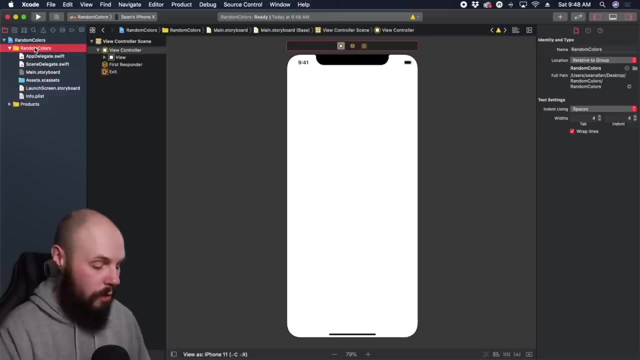 have to be connected to a file. Remember we had that view controller file. They were automatically connected. Again, I'm going to show you how that works. So in your random folder- colors folder- do command N to get a new file. 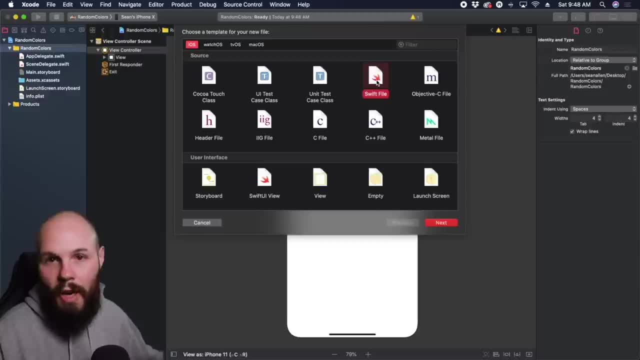 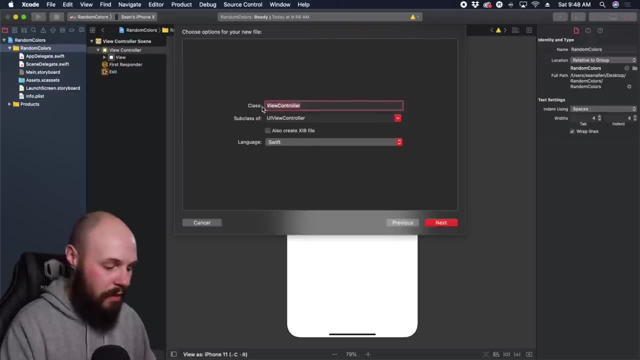 Cocoa touch class. Sometimes we'll do swift file, which is just an empty swift file And we have to type everything ourselves. We're going to do Cocoa touch class So that'll fill in some of the boilerplate code for us. I'm going to name this: colors table VC. 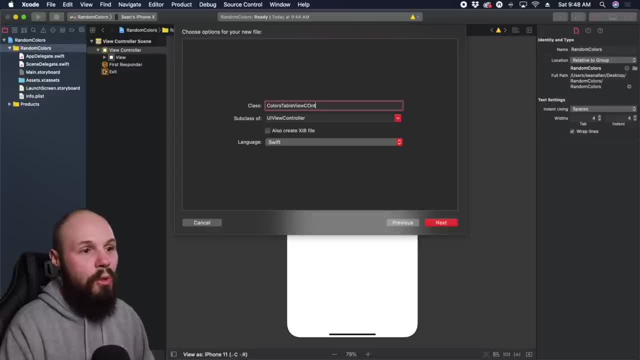 Now I'm doing VC, short for view controller. Some people will type out view controller every time. As you can see, that just becomes a really long name. I think it's also redundant. I just do VC. That's a personal style choice. 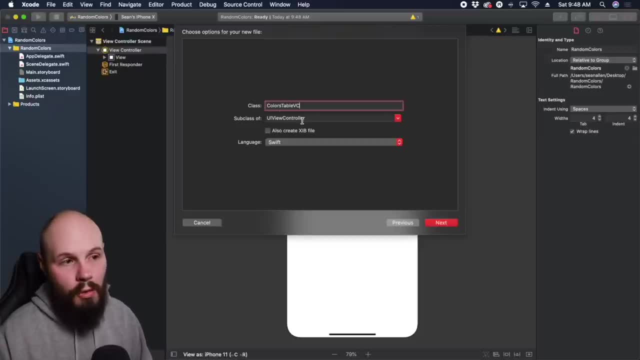 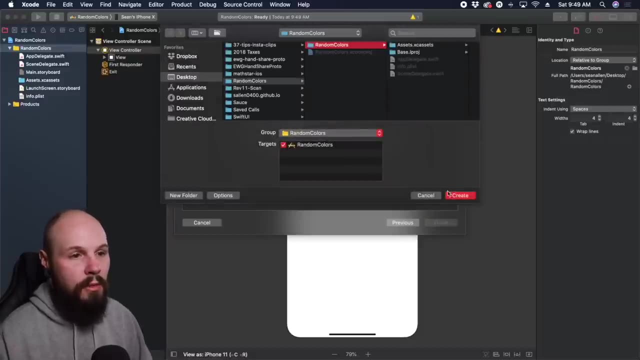 Name it whatever you like. You can see subclass of UI view controller. That's what we want. We don't want to create the zip file and then the language is swift, So hit next and create it in your random colors file. Now I just like to move these up. 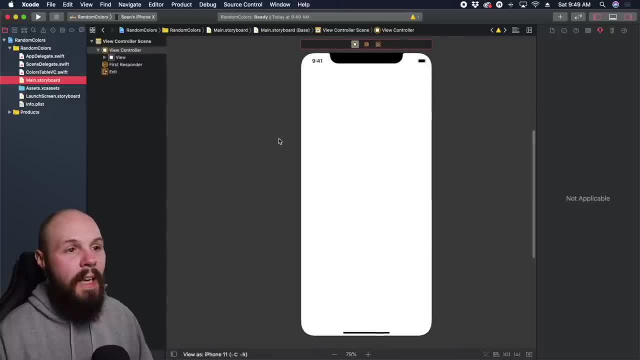 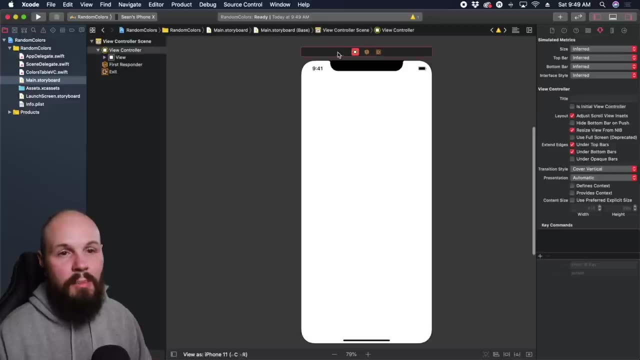 So they're all next to each other. So now, back on the mainstoryboard. I need to connect this view controller to this color table VC file. The way to do that: make sure you have the view controller selected Again. I just click on this bar up here. 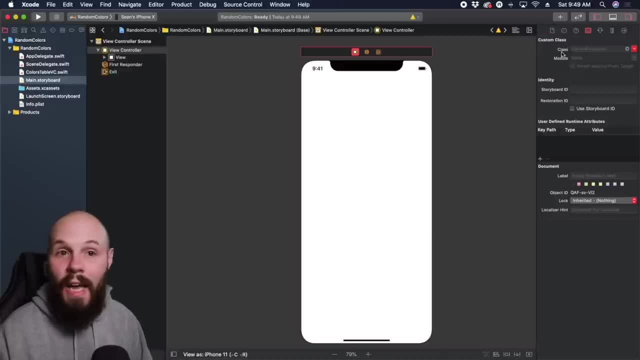 In the identity inspector, which looks like an identity card. you see class. Right now it's just the UI view controller. Well, we need to make this a colors table. VC, Hit return. That'll do that. So now this file over here. 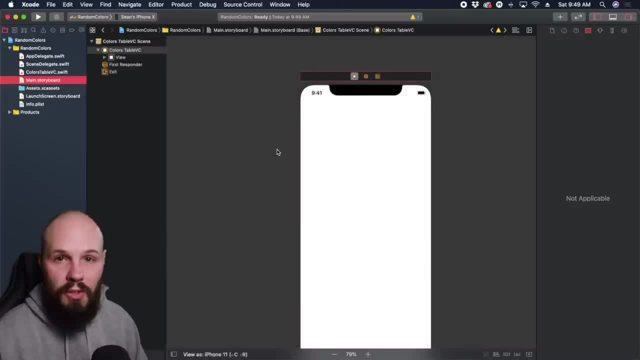 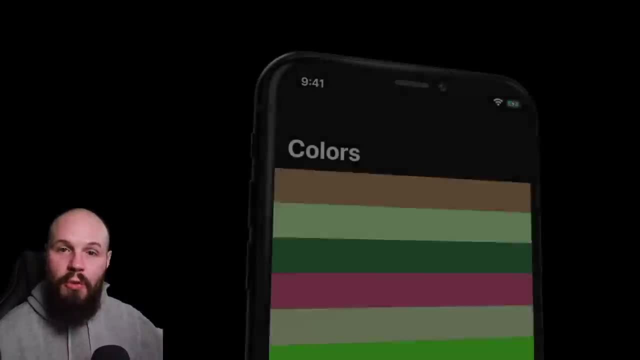 colors table VC is connected to this view controller on the storyboard And you're going to have to do that for all the view controllers that you add. So now we have the view controller that is going to become our table view that has random colors in it. 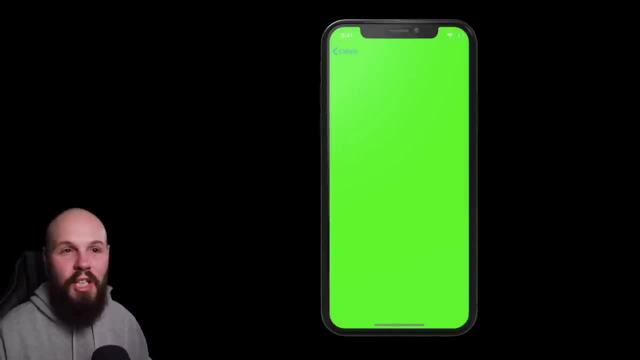 You know that won't happen for another video or so, but we need to set up the foundation, And the foundation of this app is the navigation right. We want to be able to tap on a random color and show another screen that has the background color. 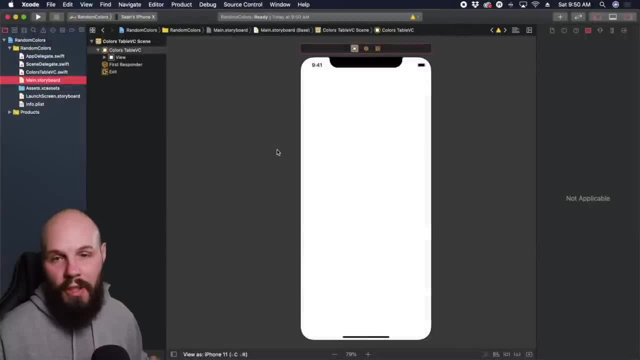 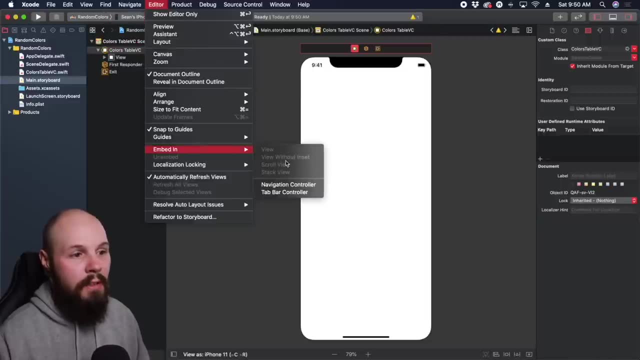 of our selected color. So to get that navigation we need a UI navigation controller. So to do that again, make sure you have your view controller selected. You can do editor scroll down to embed in navigation controller and you'll see. 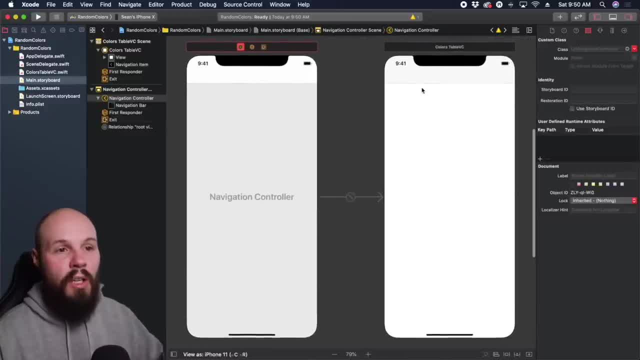 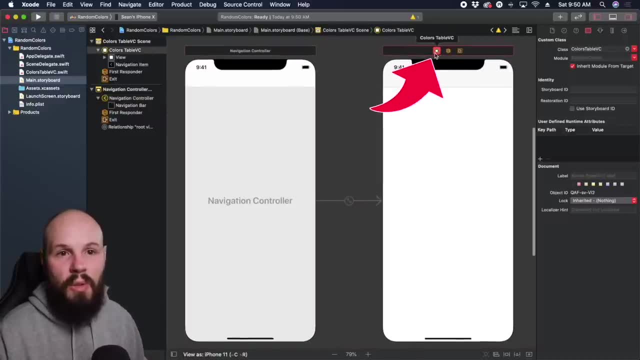 we're going to get these two up here. So you see, we have the navigation controller on the left and our colors table VC on the right. Just so we can distinguish, let's click on our colors table VC. Make sure you click on this little circle. 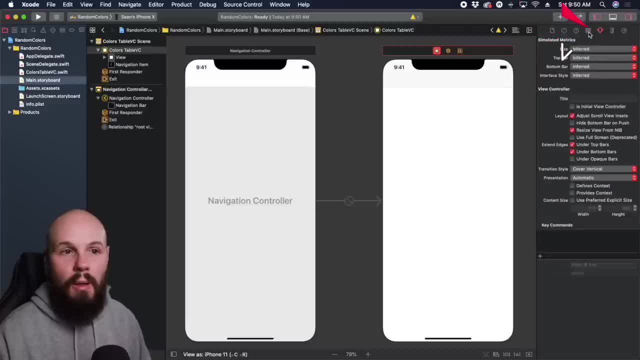 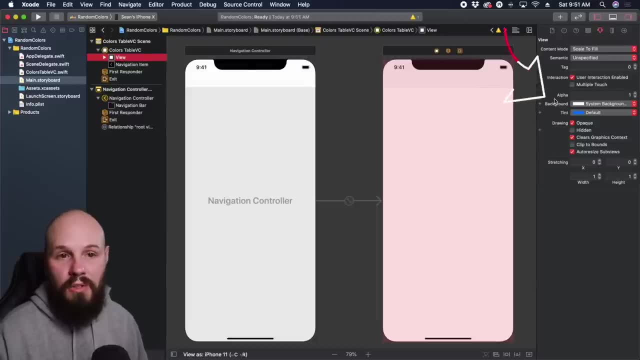 or that's highlighted In the attributes inspector. I'm sorry we have to have to click on the view, not the overall VC, the view right, Cause we're going to change the background color of this view, So, as you can see, we get background color. 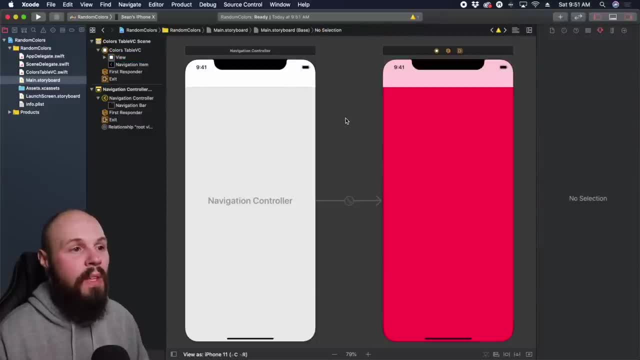 So let's make this system pink just to show that we have it. And you see, now we have a nav bar in our view controller up top. We didn't have that before, but because we're in a navigation controller, now we have that. 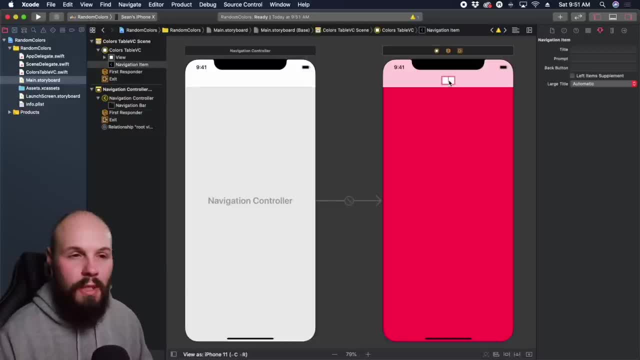 And if you double click into it, you can also do this programmatically. We'll address that later. Let's just call this colors and hit return. So now we've titled our screen colors, And before we run it, there's one more thing we have to do. 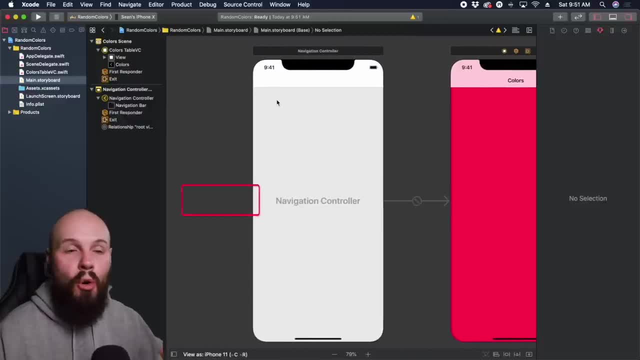 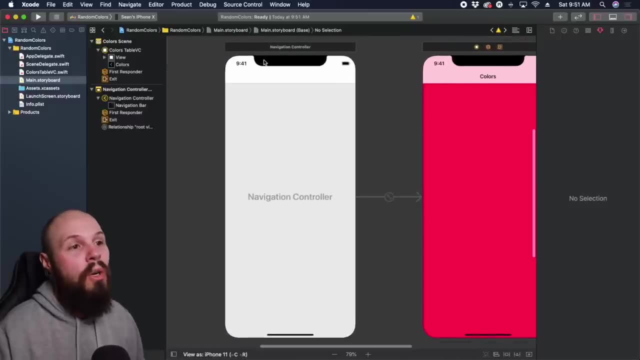 Remember that is initial view controller. right? Xcode needs to know what view controller to show first, right, Cause right now we just have these two things on the screen. Xcode doesn't know what to show first, So we need to show the navigation controller first. 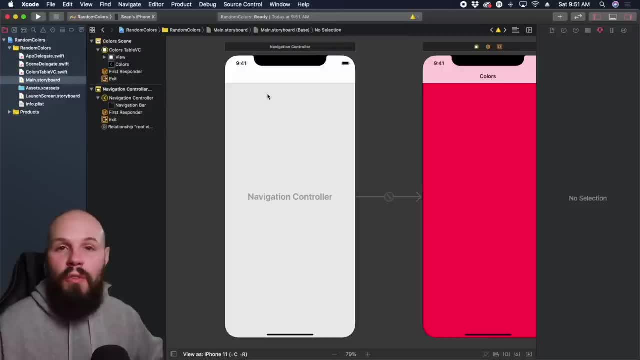 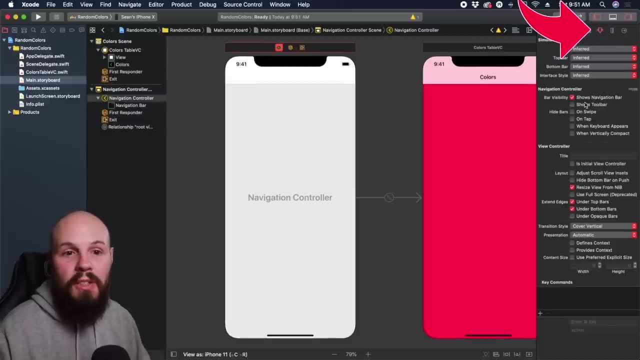 because the navigation controller is a container that holds all of our view controllers. We'll get into that in a second. So click on your navigation controller and then over here in the attributes inspector, you can see down here is initial view controller. So by clicking this, you see, we get this arrow here. 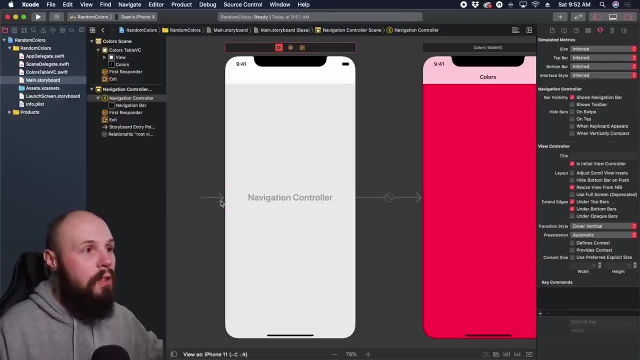 So this is telling Xcode. hey, this is the first thing you need to show. So let's actually run this so you can see that in action. not on Sean's iPhone X, just run it on the iPhone 11 Pro. run it. 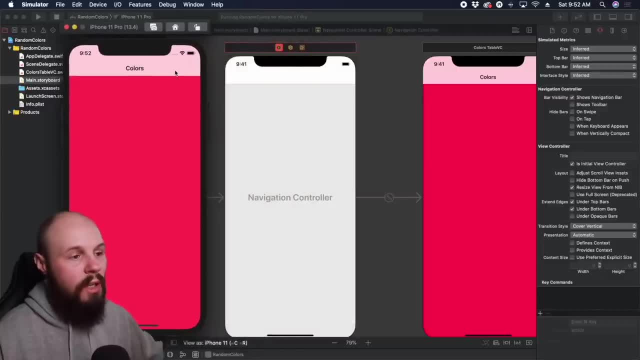 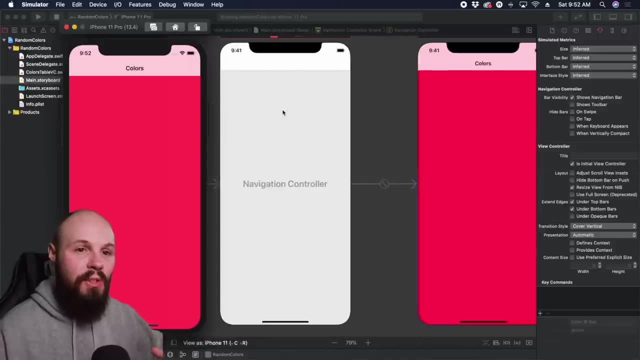 And here we are. you can see we have the colors app with the nav bar up top. So you can see the navigation controller is a container that holds this. Let's actually build the next screen before I dive into how the navigation controller works. 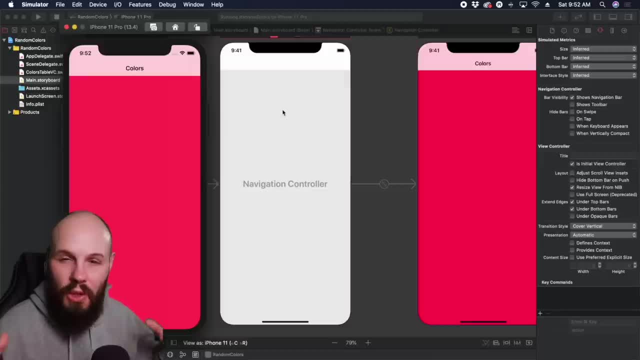 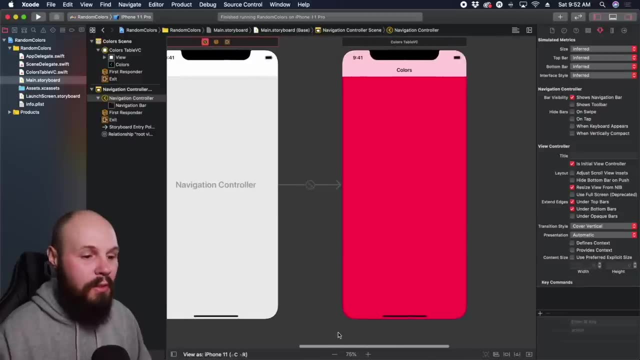 That way I can actually show it to you on the simulator, and it'll make more sense when you can see it in action. So let's stop this and zoom out a little bit. Well, you may not have to again, my resolution is just huge. 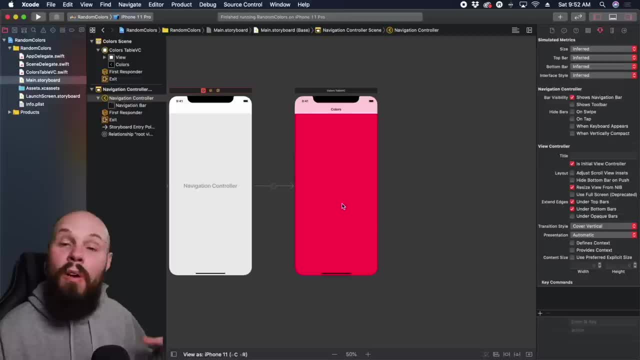 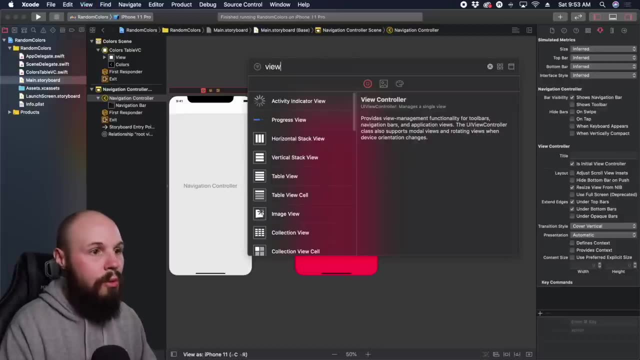 So we need to add another view controller onto the screen Cause, remember, this pink screen is going to be our table view that we're gonna tap on and show the next screen. So let's do command shift L type in view controller, hit return. 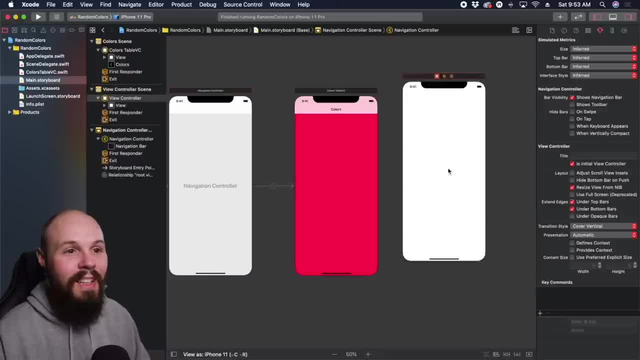 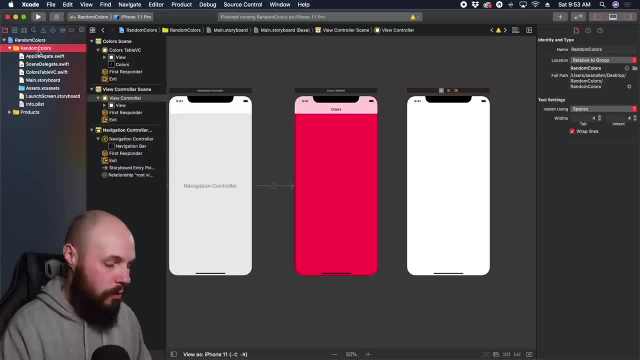 tap on the screen or double click on that or drag it- Jeez. So now we have this other view controller. again the same process. We have to attach this to a file. So in our random colors folder, do command N for a new file. 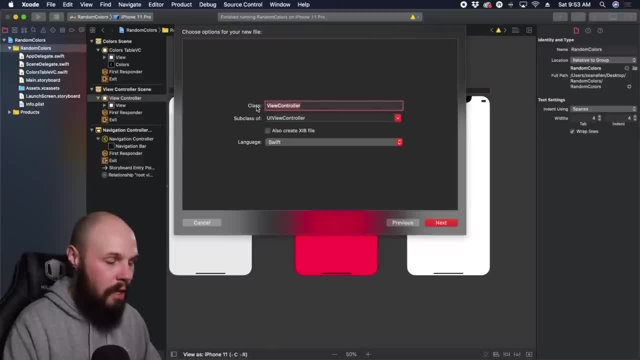 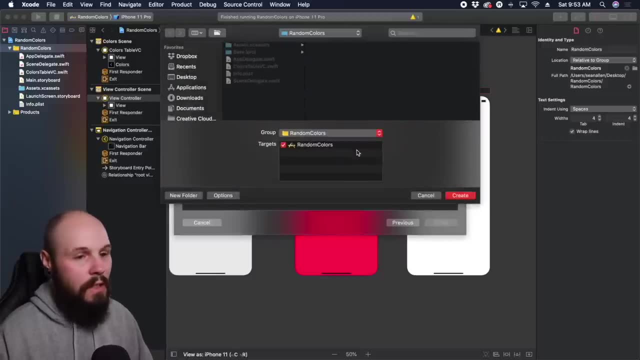 Cocoa touch class hit. next. We wanna name this the colors detail VC and it is subclass of your view controller Swift. Next, save it into your project. Here we have the code Again. I like to just drag this up, so they're there. 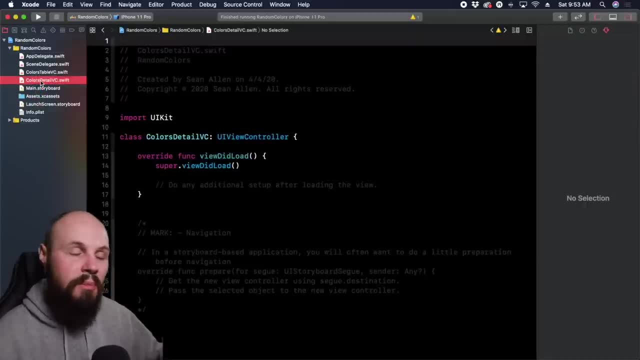 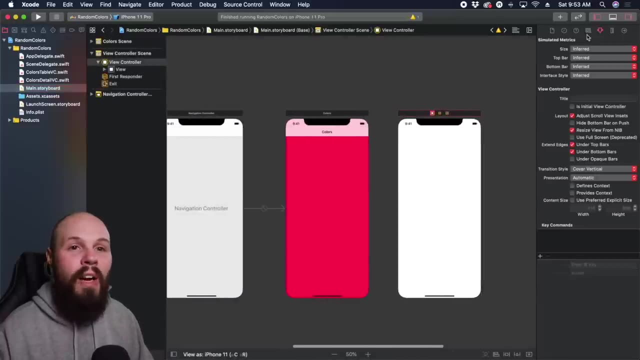 In the future, as a project gets bigger, you know you'll create a folder structure. We're not gonna dive into that now, but back to our storyboard. Now we need to attach this new view controller that we've added to that file. 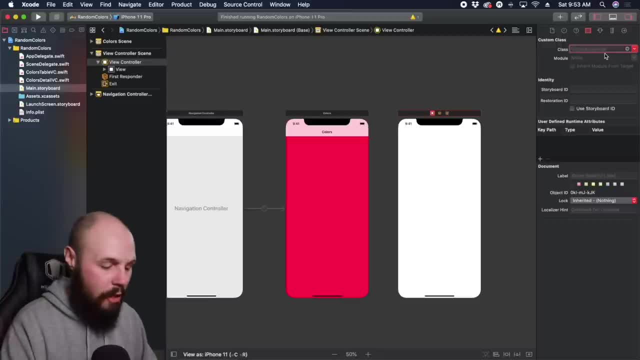 So again, the identity inspector. the class is just blank right now. Let's name it a color detail VC. Make sure you hit return Again. if you don't hit return, it's not gonna connect it. I've made that mistake before. 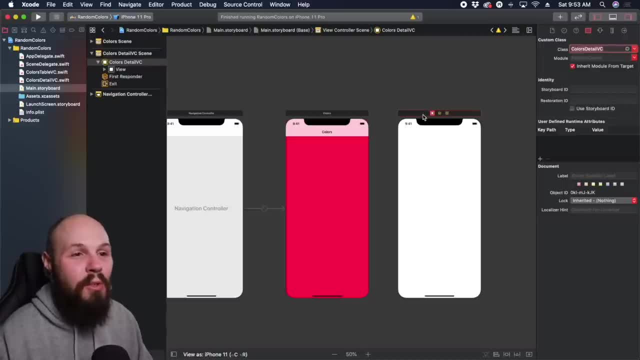 I'm sure you will too in the future. Hit return. There we go. Now this view controller. right here is a color detail VC, but you'll notice we don't have a navigation bar up at the top. That's because it's not in our navigation controller. 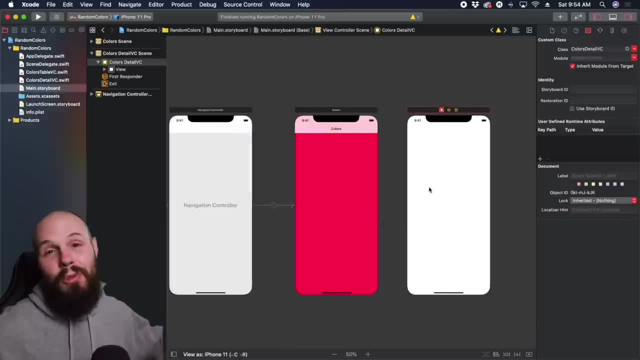 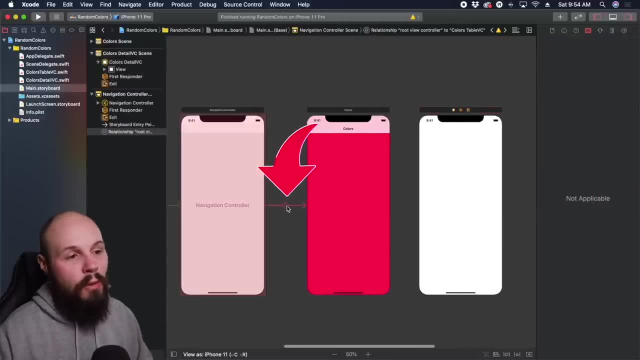 Right now, this colors detail VC is just a random view controller floating in the abyss Right. We gotta put it into our navigation hierarchy. So what this is called right here, this is a segue And you can see our navigation controller has a segue. 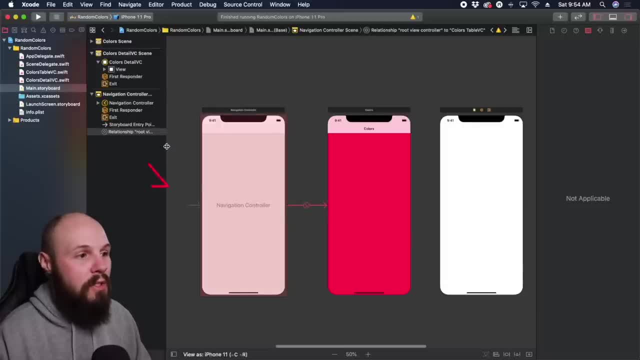 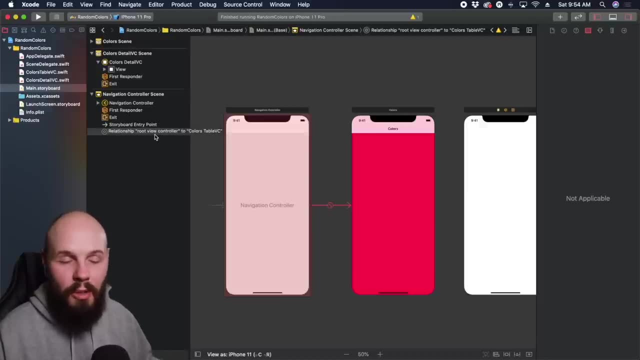 to this colors view controller, And this is a special segue. As you can see over here, it is a root view controller. So remember, a navigation controller is just a container And again, I'm gonna explain this more in a bit. 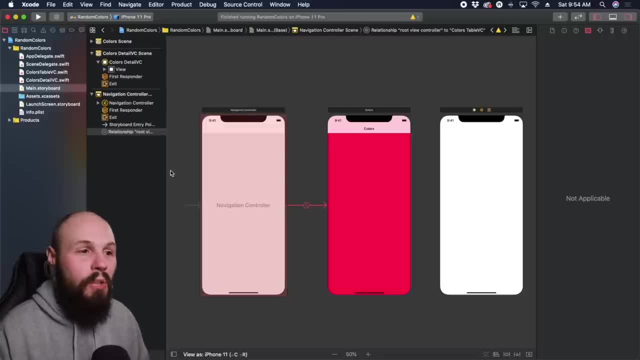 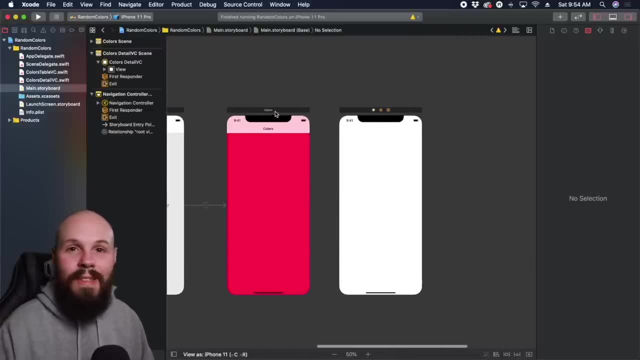 So, since it's just a container, you have to tell it it's initial thing that it's holding, or else you won't see anything. And right now it's holding this pink view controller. That's the root view controller. So now let's add another view controller onto the stack. 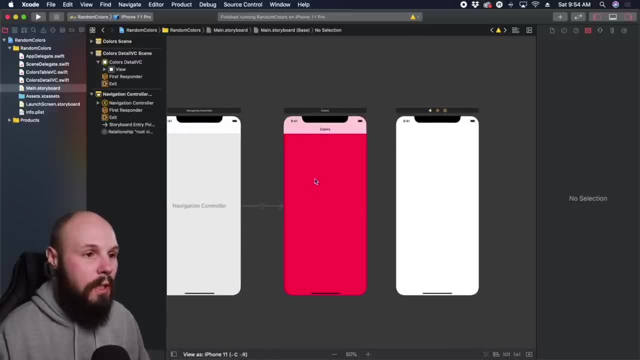 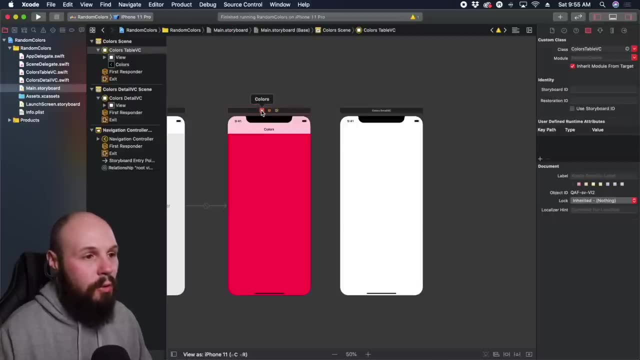 Because, again, a navigation controller holds a stack of view controllers. I'm kind of getting ahead of myself with the explanation, but let's connect this. So, if you click on this pink view controller, hold control and drag to this next one and then let go of the mouse. 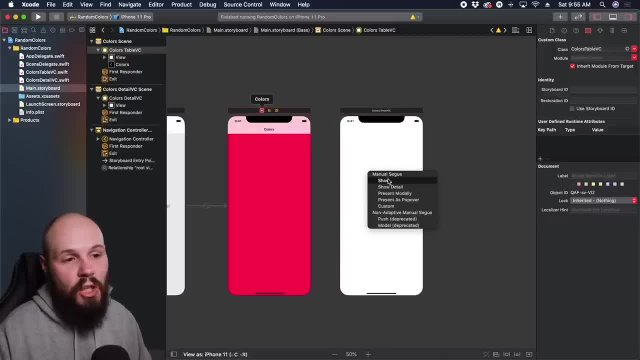 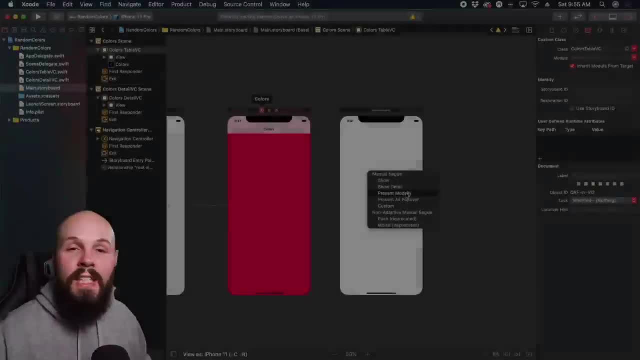 you'll see segues that you can create. So you can create a show present modally. So present modally is when it slides up from the bottom. We're gonna be doing that in a future app. That is not part of your navigation controller. 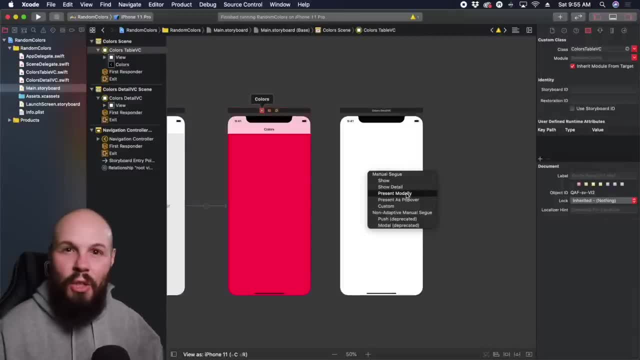 when it slides up from the bottom, It's kind of like a temporary context that shows and then you swipe it down and then you're back to what you were doing. Do a show segue. that will put it in the stack of view controllers that the navigation controller 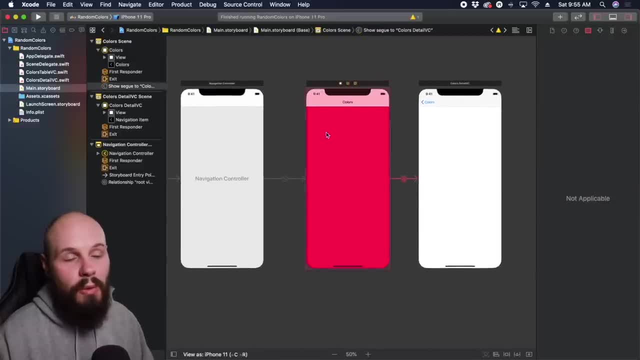 is holding. So now we have this segue from the pink view controller that we have here- our colors table VC- to our colors detail VC. We need something to trigger that segue, And real quick. if you click on the segue, we have to name this. 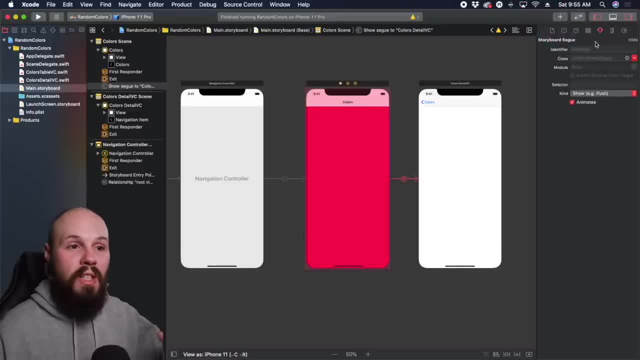 So let's go to the attributes inspector, because what we're gonna do is we're gonna say, hey, fire off the segue named this, So Xcode knows what segue to use. So here in the attributes inspector, having your segue clicked, name it. 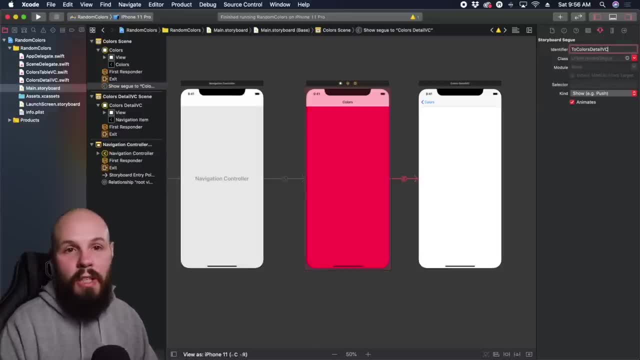 We're gonna say: two colors, detail, VC, hit return. Again, make sure you hit return. So now we've named our segue, so we know how to access it. So now we just have to have an action to trigger that segue When the app is fully built. 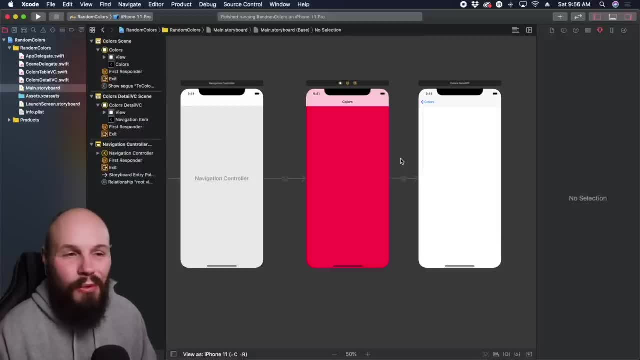 that's what's gonna happen when we tap on a cell. However, we don't have our table view set up, So we need to add a temporary button just to fire this off. We're gonna be deleting this later, but I wanna show you how the navigation works. 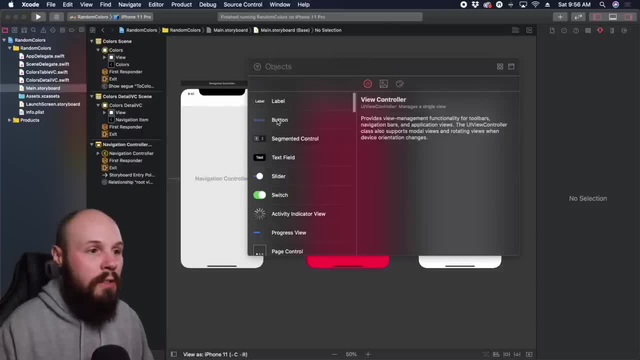 before we build out the table view. So hit the plus button. Here we have a button. Go ahead and drag the button onto the screen. Just gonna put it in the center. I'll zoom in here. I'm not gonna worry about crazy constraints. 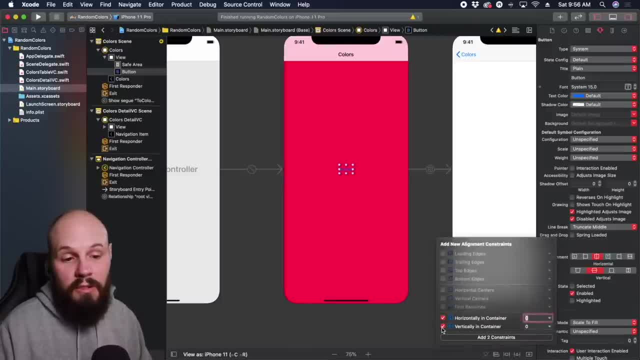 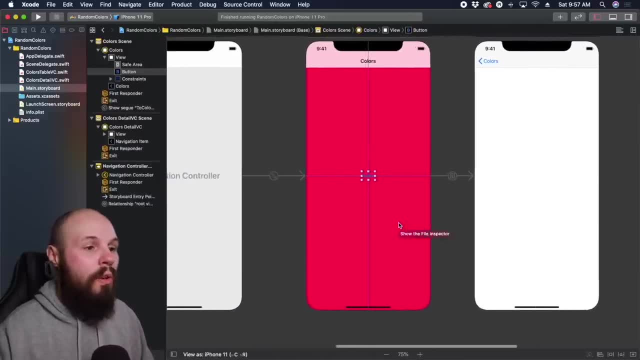 So here in the alignment I'm gonna do horizontally and vertically, in container hit, add two constraints. So now we're gonna introduce you to outlets here. So in order for items on the screen to be able to be used in the code, you have to create what's called an outlet or an action. 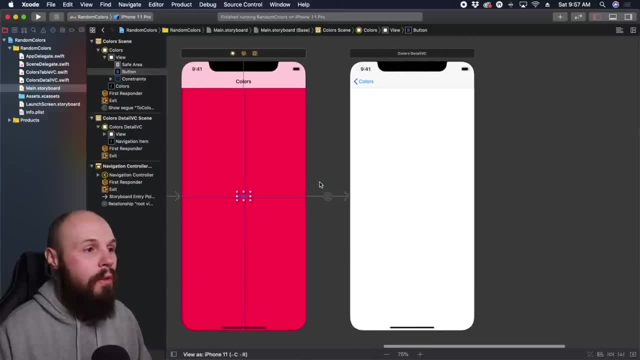 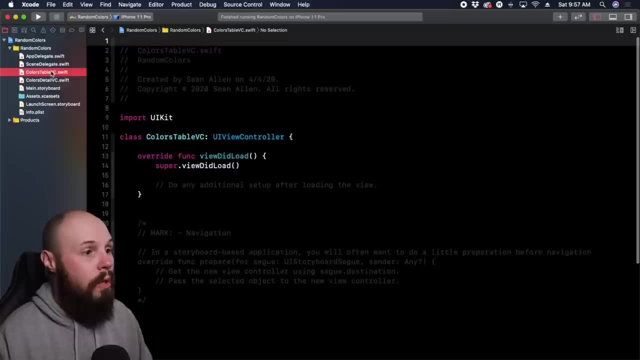 So here we're gonna connect this button to our code, So I'm gonna move it over here And in our colors table VC, cause, remember, that's the code that's attached to this view controller. So here's our color table VC. Whoops back to the main storyboard. 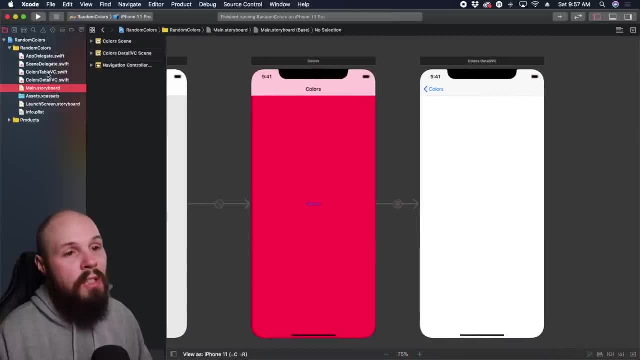 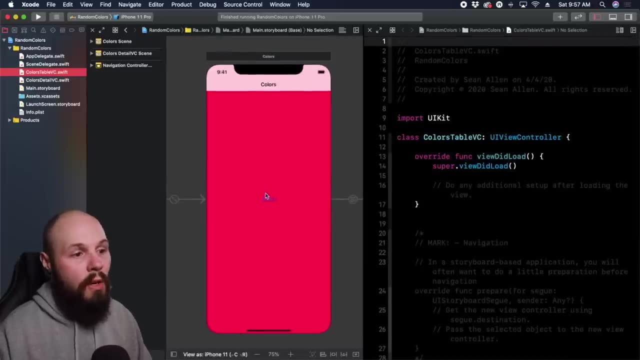 If you hold option and click on the colors table, VC, it'll pull up your assistant editor right. So here we can have the storyboard on the left and then our code on the right for this screen. So now, if I click on the button, 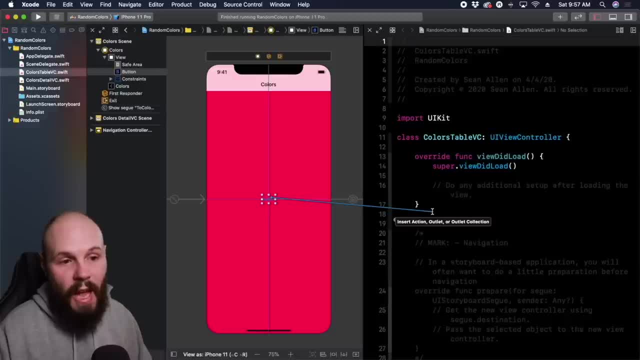 if you hold control and drag, you can create. you see insert action outlet. We wanna insert an action, So you see the connection is already in action. The object is colors. That's the title of the screen we're on, So we wanna name this. temp button tapped right. 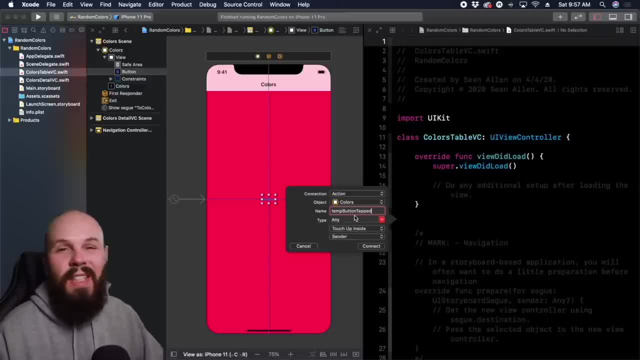 That's what happened. That's the name of our action Whenever our temporary button is tapped. this is the name of the function, pretty much. The type is a UI button and touch up inside is the default and sender is the default. that's fine. 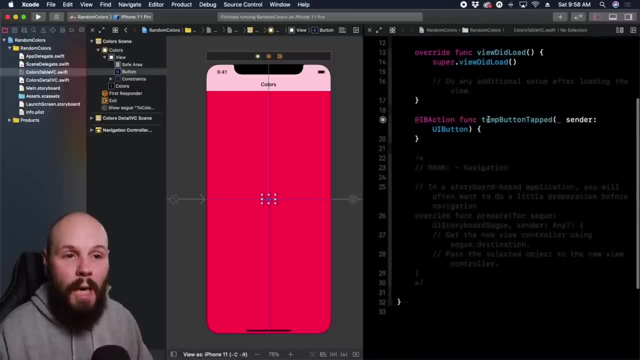 So hit connect And now you see we have this code over here, A temp button tapped, So whenever our button is tapped, this is the code that's gonna execute. So we created a IB action, as you see right here, to connect our interface builder. 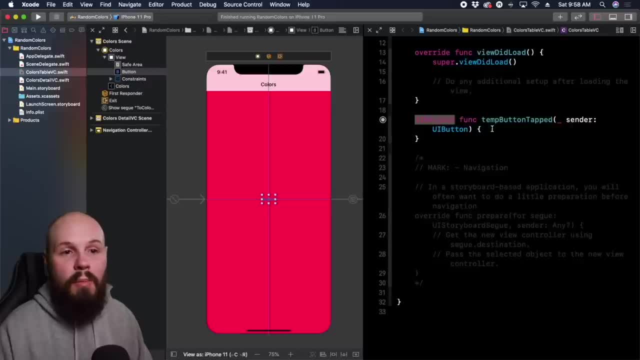 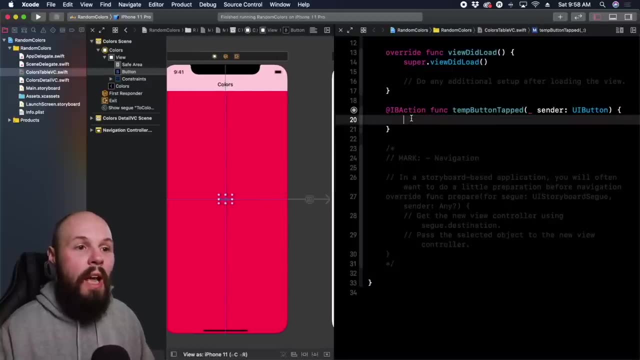 That's what IB stands for- to our code. And again, whenever the button gets tapped, this is the code that's going to execute in here, So let's execute that code. I'm gonna slide this over, So it's on one line and it looks nice. 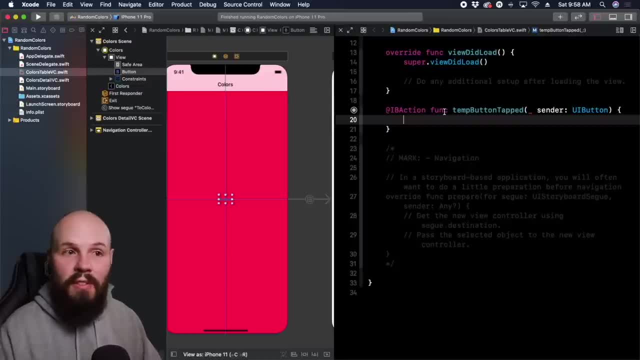 All the view controllers have a perform- segue with identifier function. So if you start typing perform, start typing segue. you're gonna get the auto complete. There it is: Perform segue with identifier. Again, I'm just gonna make more room. It's gonna look a little sloppy right now. 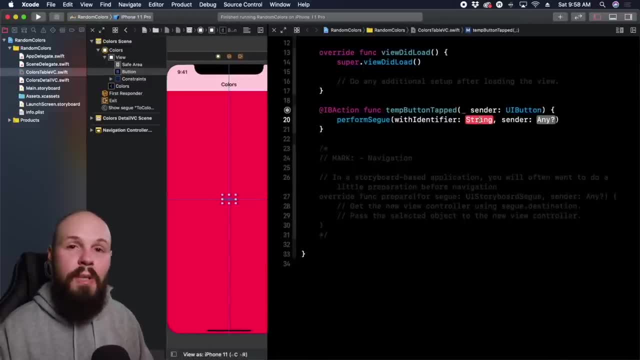 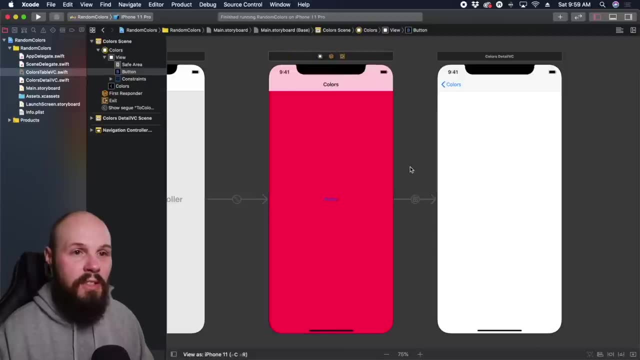 So remember, this identifier is what we used on the storyboard, Remember we named it to detail VC. So I'm gonna actually go back to the storyboard. I'm gonna close out our code real quick. hit this X And this is just to navigate around screens. 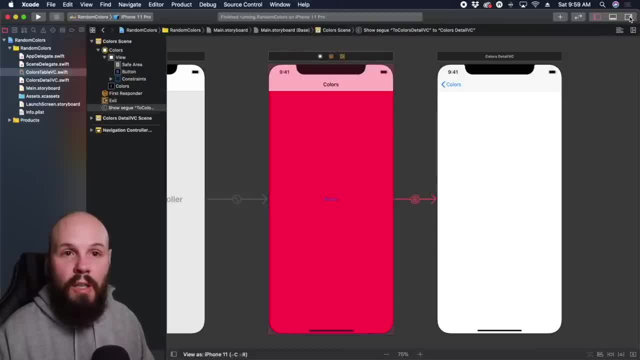 So, with this segue clicked, if you pull up the inspector, you see we got the two colors detail VC. That's our identifier. I'm gonna copy and paste this just to ensure I don't make a typo. And then now let's open up. 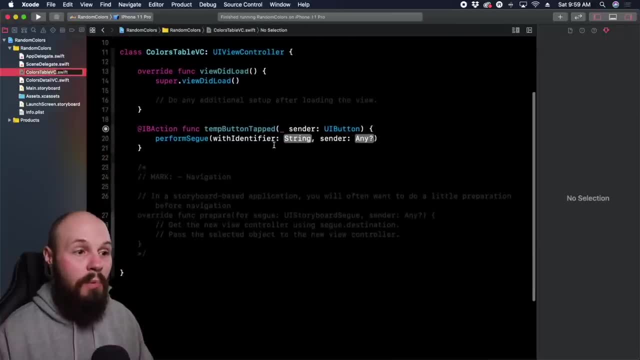 our code on the colors table VC. And now we wanna paste that identifier in right Cause. we're saying, hey, perform this VC, And it's a string, So you gotta put the quotations around it And then sender nil. 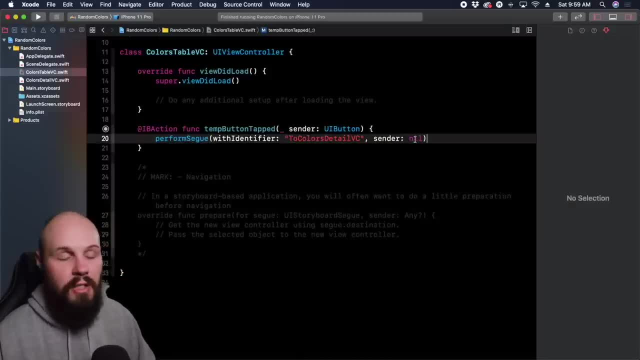 We don't have a specific sender right now. This is how you can like pass information. We're not gonna do that quite yet. So as this reads whenever our button is tapped on the screen, we're gonna perform the segue with: identifier to colors: detail VC. 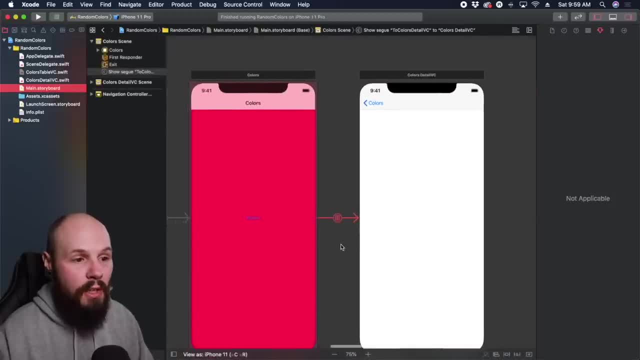 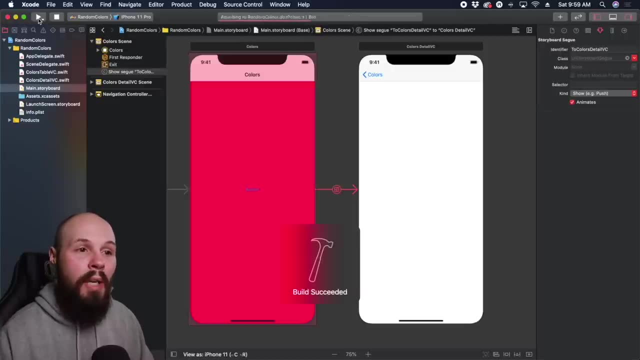 And again, that is this segue right here that we have clicked is going to be performed. So again, that's what that code does. So now let's run our app And now, when we tap our button, we should perform that segue. 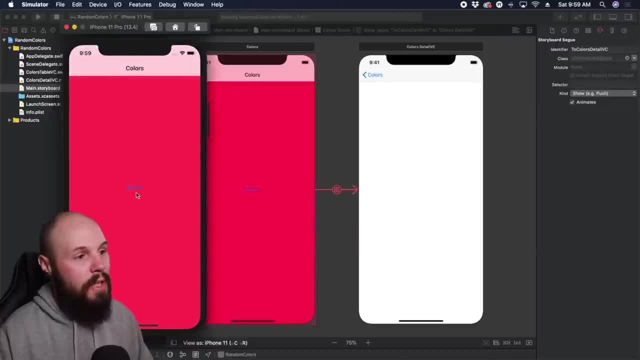 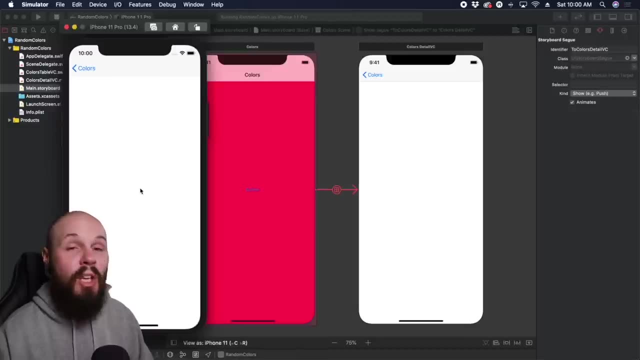 And this is where I'm gonna start explaining the navigation controller to you as well. So here we can tap our button and you can see our new detail screen slides in from the right and it's on top of our colors VC. So when you hit back, we're back to our colors VC. 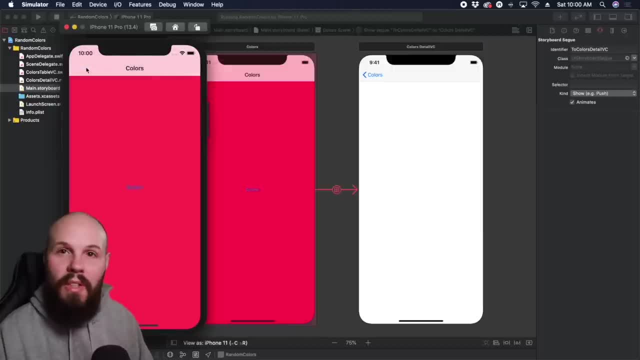 So again, button to bring in the next screen back right. You're probably familiar with this navigation. It's kind of the default navigation for apps. Now let me start explaining this. I'm gonna start explaining the navigation controller. Let me zoom out. 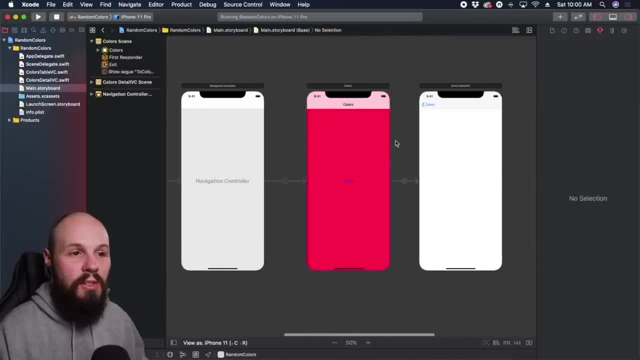 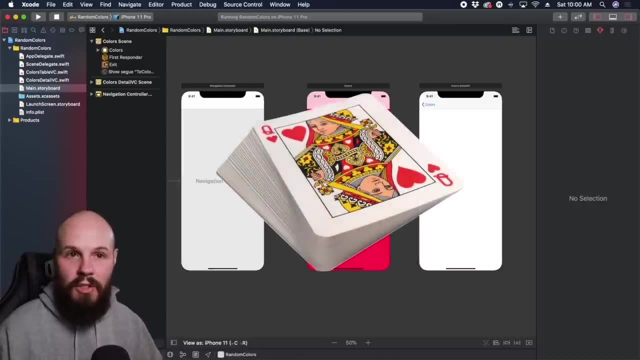 So you can see, the navigation controller is just a container that holds these two screens, And I always like to compare this to a deck of cards. Imagine your UI navigation controller is holding a deck of cards and each card represents a screen or a view controller. 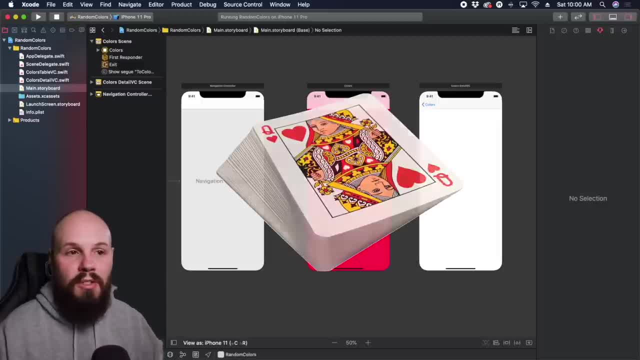 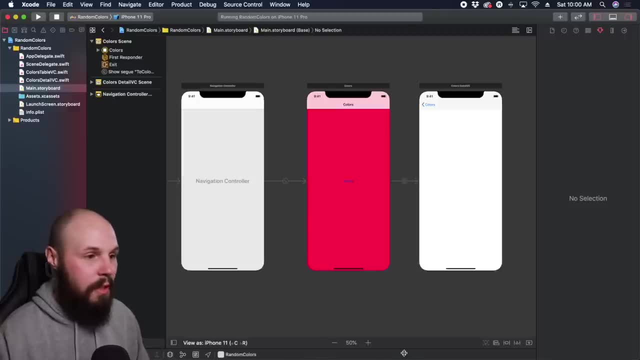 And as you add new view controllers onto the stack, you're just building up this stack of cards. So when I tap this button, I'm doing what's called pushing a view controller onto the stack. So again back to the simulator. So right now, my navigation controller, stack of views. 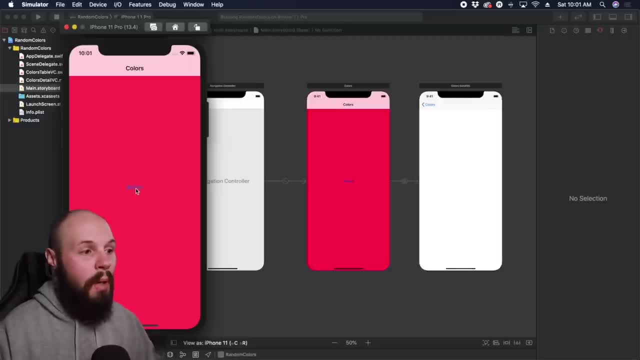 of screens is just holding the pink screen. When I tap the button now we're pushing a new view controller onto the stack. So right now my navigation controller is holding a stack of screens. At the bottom of the stack is the pink screen. 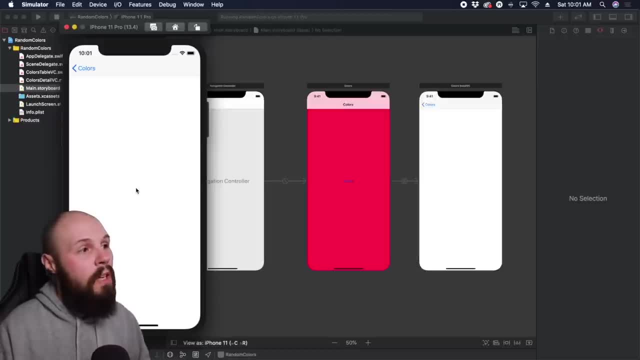 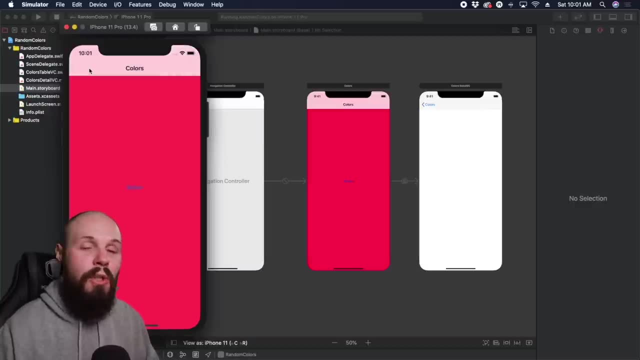 on the top of the stack is the white screen that you see here. So now, when you hit back, what you're doing in the navigation controller is you're popping that top screen off of the stack to reveal the bottom screen, And then again. 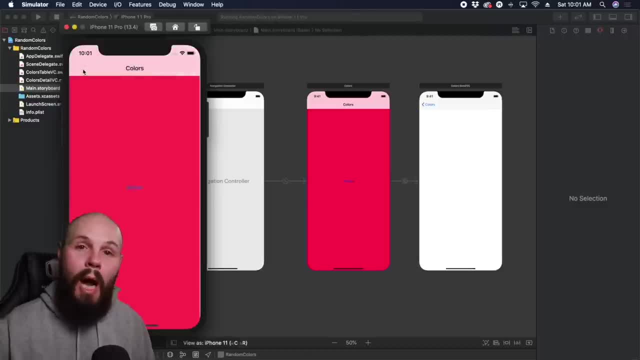 now we're adding that white screen back on top of the stack And here when I tap back we're popping that off the top of the stack. So again, if you kind of visualize this deck of cards or a stack of cards, 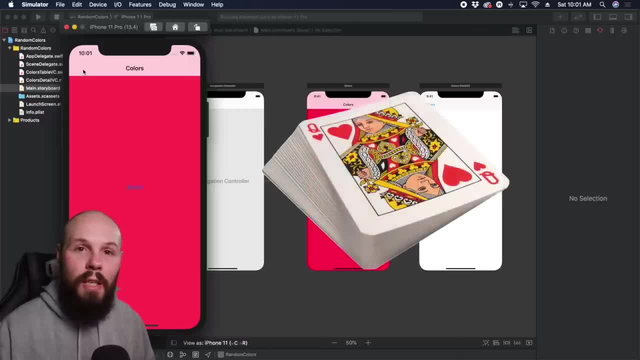 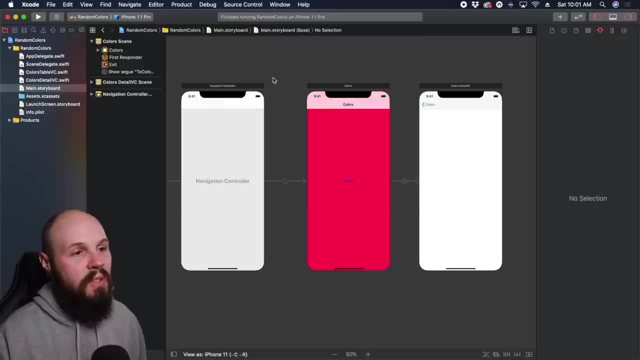 and those are like your screens. all you're doing is adding new cards onto the stack and popping ones off the stack. So that's the fundamentals of how a navigation controller works. I'm gonna stop this. We're gonna do one more thing to customize this a little bit. 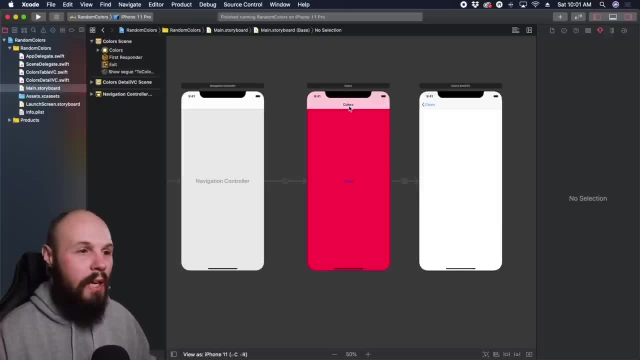 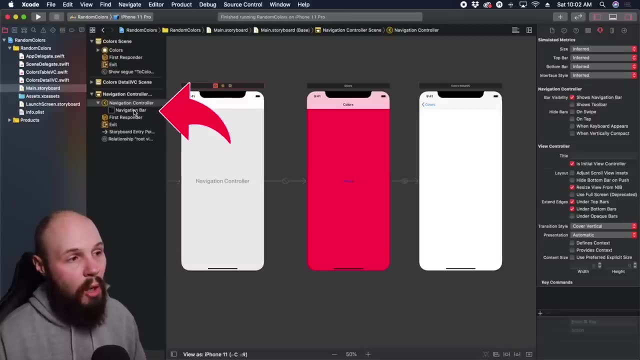 If you notice, this is like the old way. we don't have those nice new large navigation titles. So here, if you click on the navigation controller, you see the navigation controller here has an item called the navigation bar. Click on that. 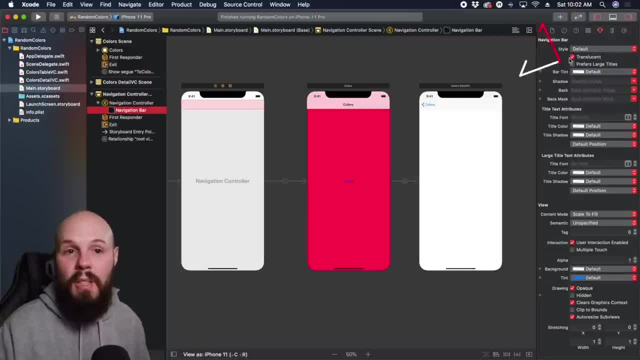 And here we can customize that in the attributes inspector. So here we see: prefers large titles. Click that And now we're gonna get the large title when we run it And you already see it on the screen right here. That is the more modern look of the app. 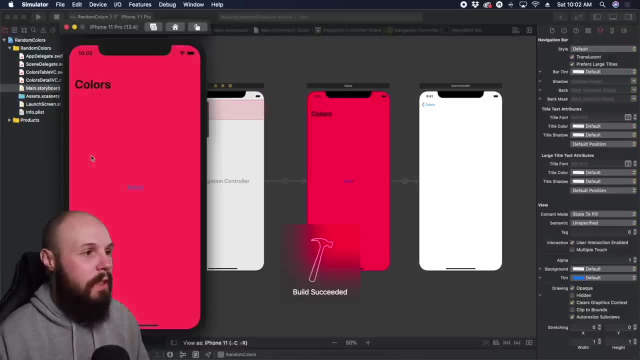 So now, when we run it, you'll see that that's what we get right. Colors, that's the more modern look Button. and then you go, you get that animation up into this back button for free. Do you see that little cool animation? 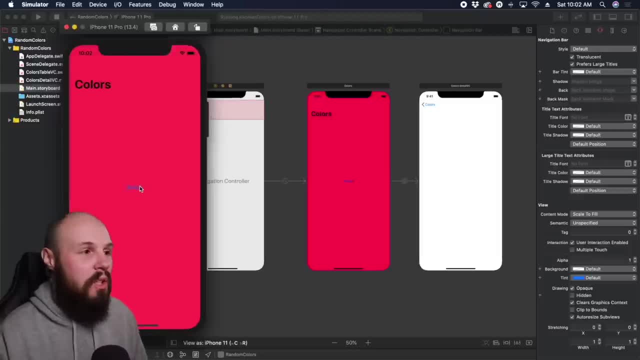 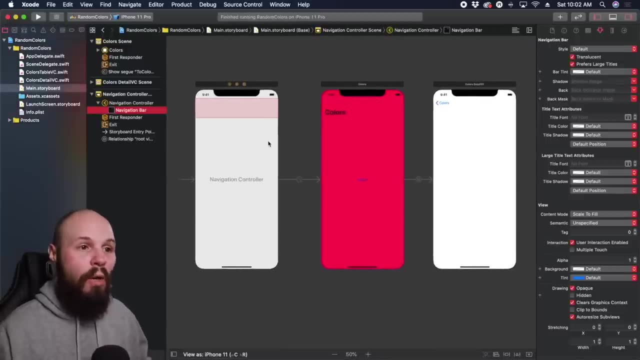 how it animates back and forth. There you go. You get that for free by using the large titles. So that is the basic navigation of our app. We have all that set up. Again. we're going to turn this pink view controller. 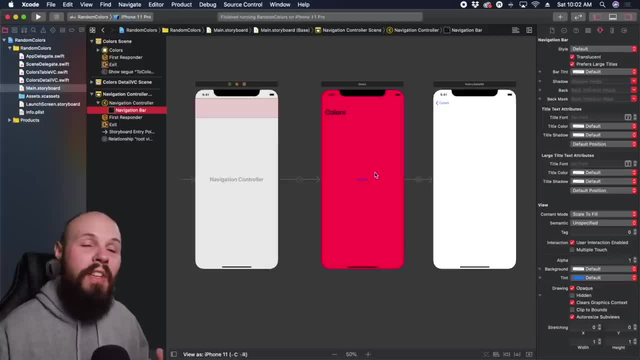 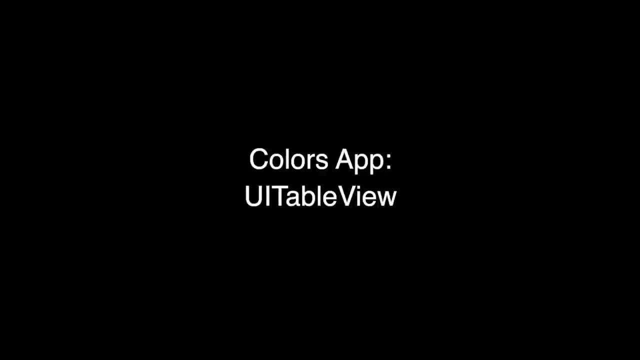 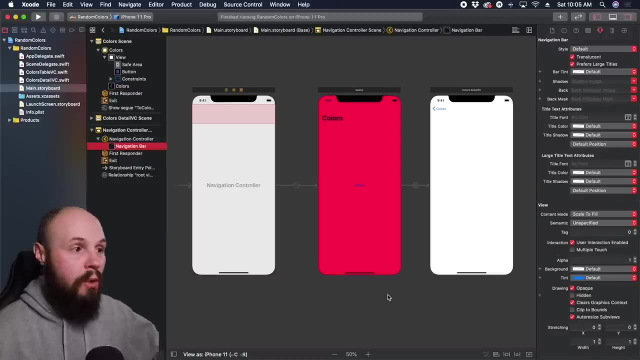 into a table view in the next video And then in the video after that we're gonna write all the code that does all the logic to finalize the app. In this video we're going to get the basic table view set up. Now, here you are, looking at the project. 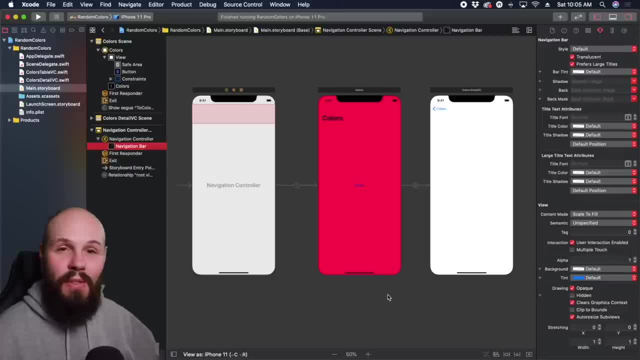 Hopefully it looks familiar. I left off exactly where the last video left off. I didn't do anything in between. You're looking at exactly where the last video ended. Before we dive into our table views, though, I want to clean up some of the temporary stuff we did. 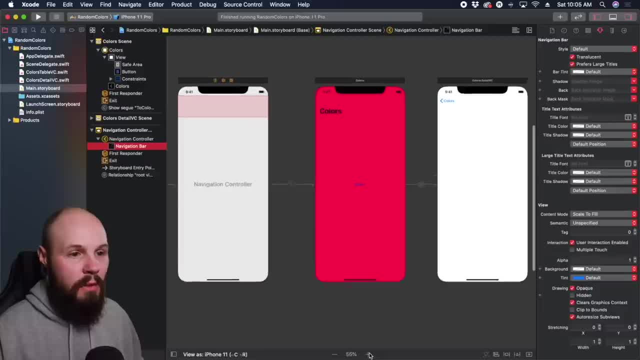 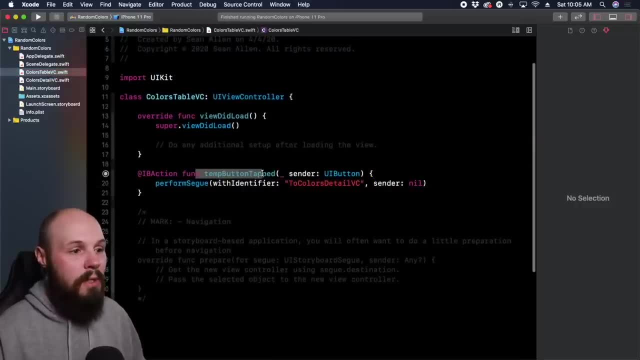 and also give a little side lesson. So let's get rid of this button here because again, that was temporary. So if you remember, in our table VC we have this code here right, Temporary button tapped. Well, here's the tricky thing with outlets, right. 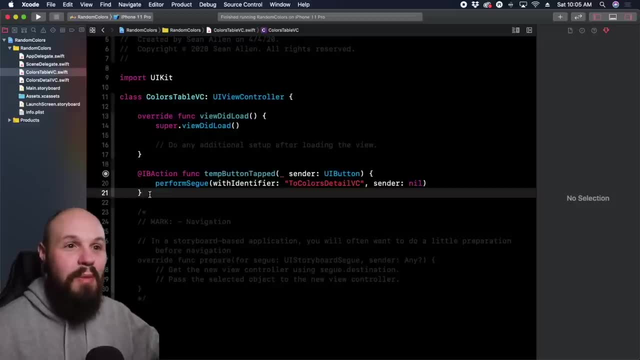 You and this is going. you're going to have this happen, right, And sometimes people will search forever because they forgot to delete like an outlet. So what happens is if you just delete this code, right, You may think cool. 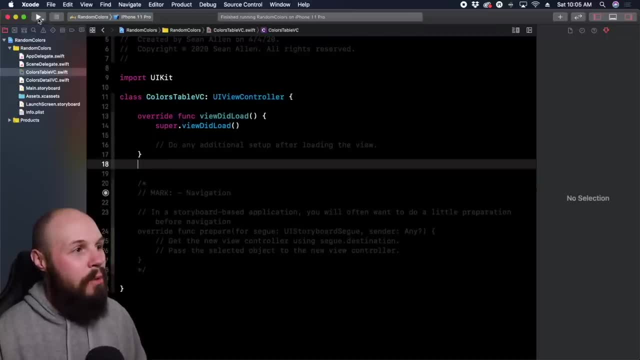 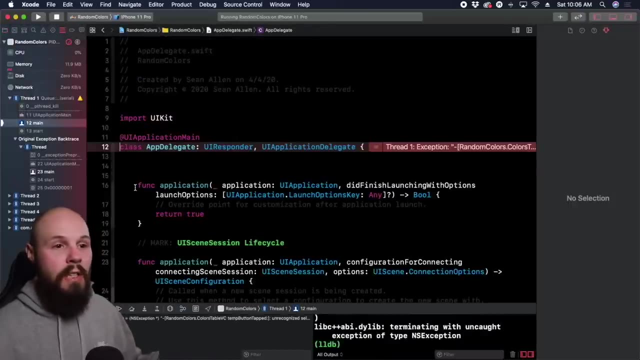 Okay, I'm good, I'm good to go. But now watch what happens when you run this. Like you may think you've deleted the code that creates your outlet, But if I tap the button, oh man, crash And it's because you've deleted one half of the equation. 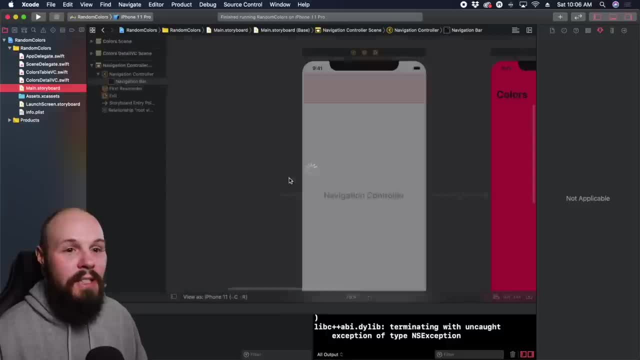 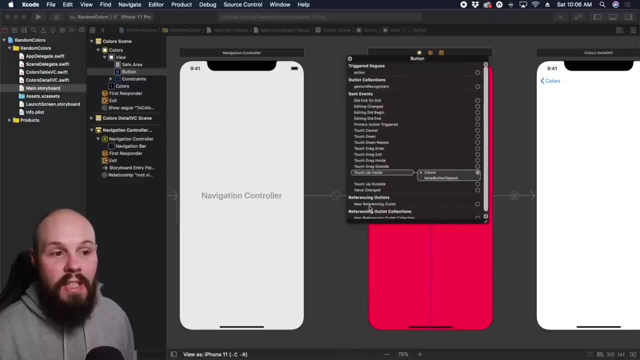 right Our button still has. let me go back to the storyboard- still has an outlet attached to it. So if I click on the button and you can see them by right clicking and you can see, this has a touch up inside outlet. 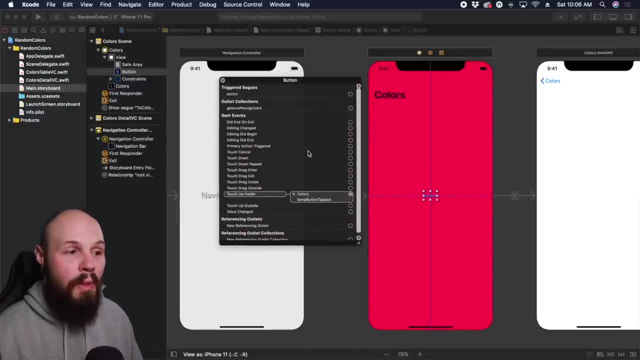 So what's happening is, even though I deleted the code, when I tap the button, this action is still firing off. So I guarantee you you're going to have crashes because you, you know, we'll deleted the code and you know. 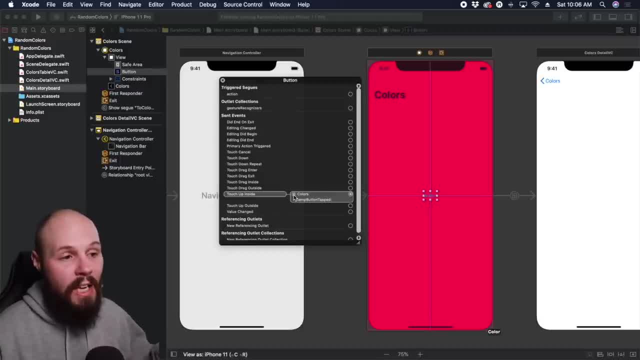 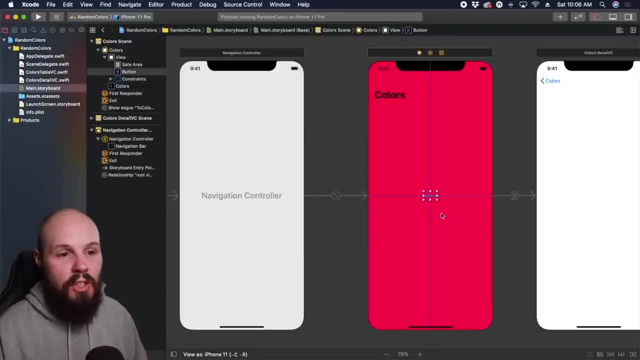 you didn't fully delete them. So you have to hit this X button to get rid of this action, to get rid of that outlet. So now, once you delete that, now you can, you know, finish everything off. Well, I guess, just deleting the button. 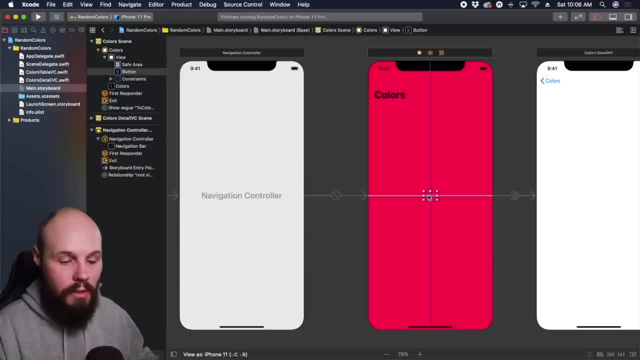 would also have taken care of that. But oftentimes, you know, you may just want to delete the action there. So now we can delete the button and get rid of that. So again, just keep that in mind. That is one tricky thing with outlets. 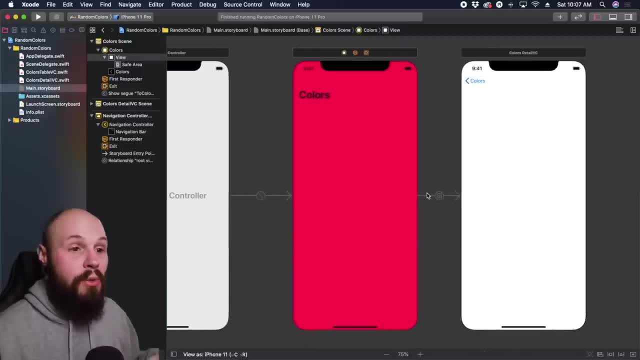 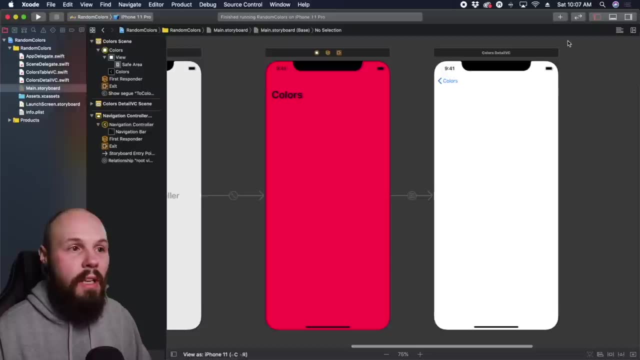 is you have to delete like both sides of the equation, meaning the actual storyboard, implementation and also what's in your code. So, okay, we've gotten rid of that. Now let's take our colors, VC and click on that. click on the view. 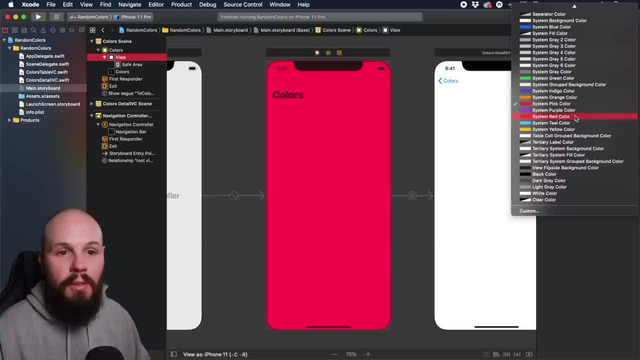 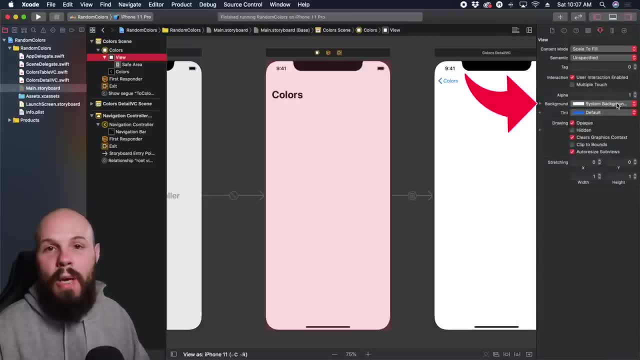 because we're going to get rid of this pink background here. So background is going to be just system color, system background color, So the system background color. if you use that rather than just white, that's what will change to black and white. 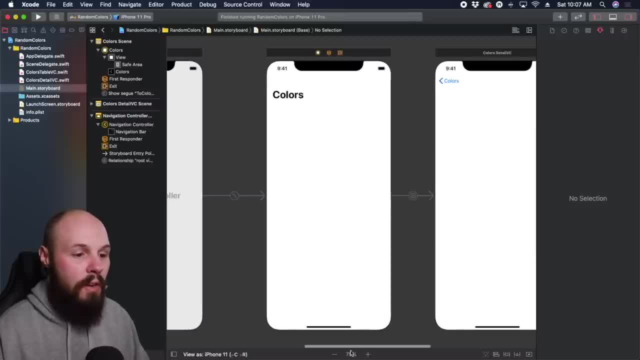 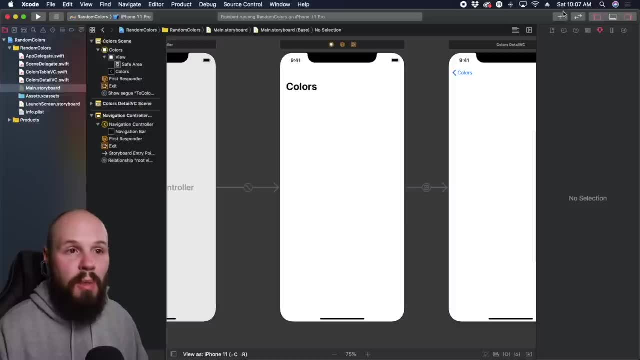 if you go from dark mode to light mode automatically. Okay, so here we just have our basic app. Now let's start building our table view. So to do that, let's actually zoom in. here again you can hit the plus button. 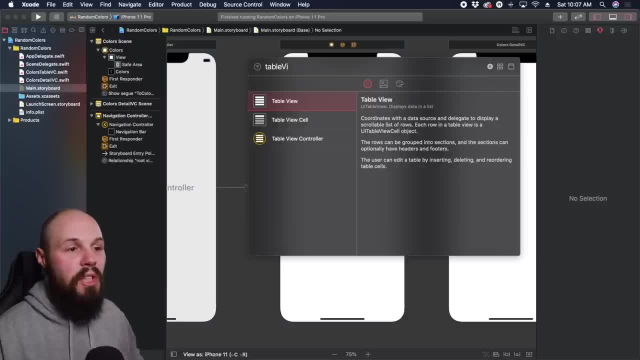 type in table view. Now you see, you're going to get a table view controller. This kind of does a lot for you. However, I'm not a fan of these. You may see some tutorials out there if you're searching for table views. 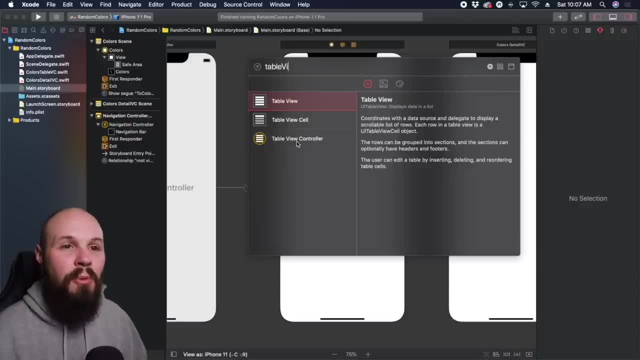 that use a table view controller, because a lot of the stuff is done for you. However, what I found in my experience is that they are extremely restrictive. If you want to create anything custom with them, it's just a pain in the butt. 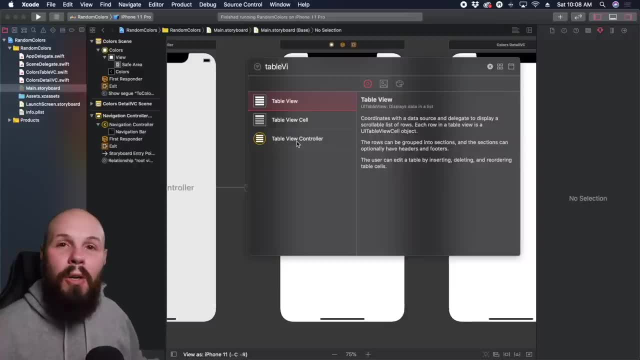 So I always take the extra minute or two to build my own custom table view. That way I have all the freedom in the world, right, I'm not like restricted, just my take on it. You may hear differing opinions, but anytime I've tried to use a table view controller. 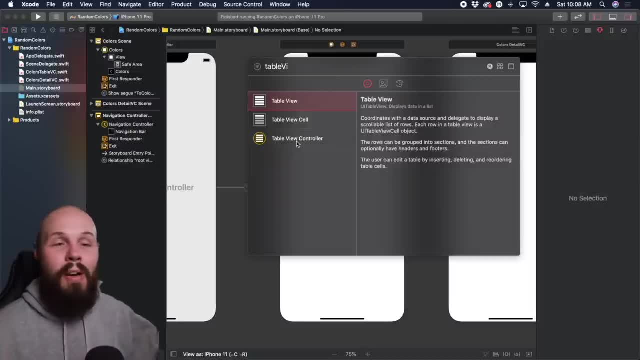 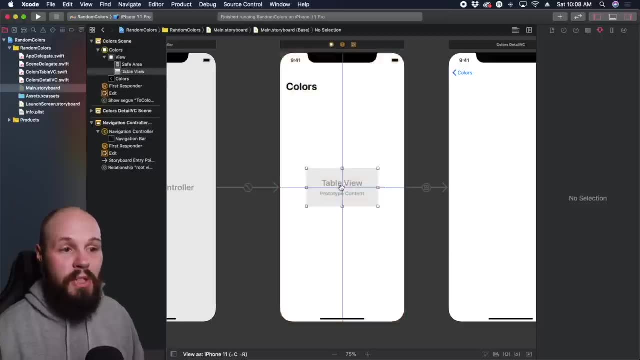 I've regretted it, So we're going to do it the custom way. so you have the freedom. So here we want to take this table view, drag it onto here and you see, we're just going to get it there. Now we want to constrain this to the full screen. 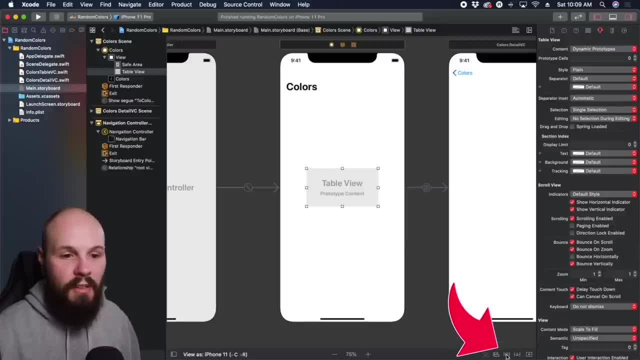 So by clicking on the table view, so we click on our TIE fighter down here and we don't want to constrain the margins. Make sure we click that off, because we don't want to have a built-in margin. So here we want to constrain it to the view. 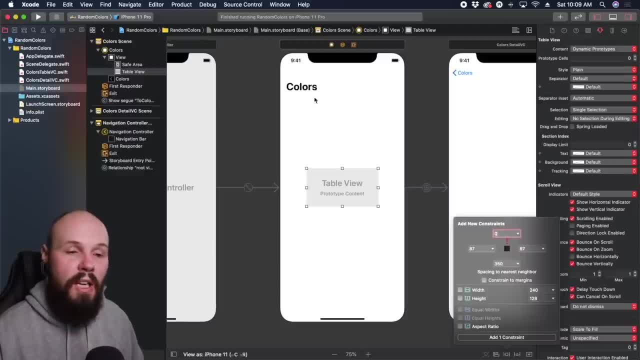 which is going to be zero. We want it to pin it right to the bottom of this colors navigation bar. Same thing here: view zero. And again, we're not messing with the safe area, So make sure you hit view zero. 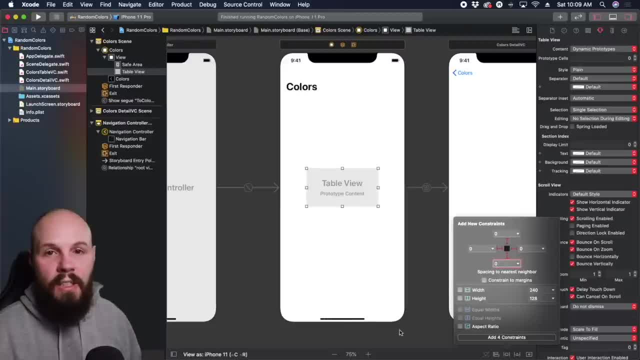 because on the bottom the safe area would be right above the home button indicator and our table view would just stop right above the home button indicator And just we want it to look like it fills up the whole screen. You'll see what I mean once we have this built. 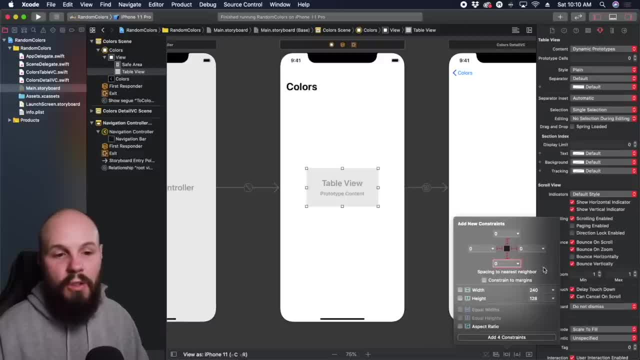 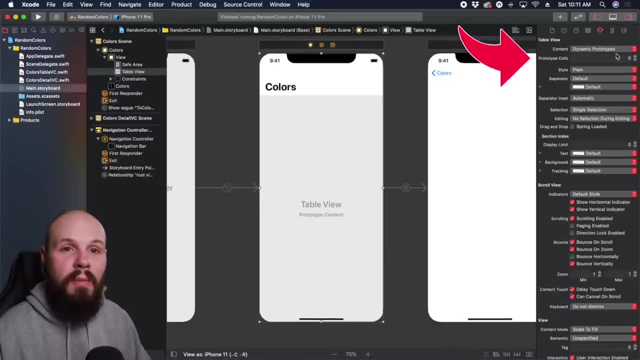 and I'll try to remember to point that out. So once you have all four of those constraints, no constraint to margin is clicked. hit add four constraints and you can see it filled up the whole view. That's what we want. And then, with our table view selected, 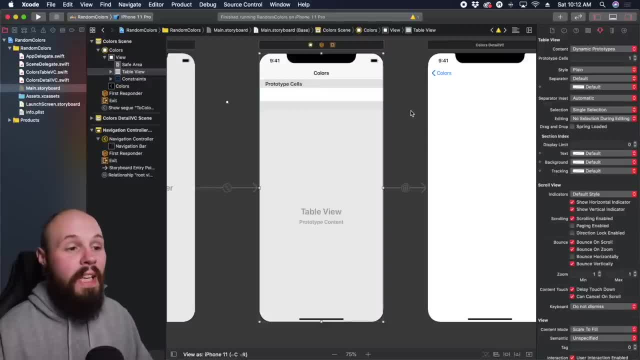 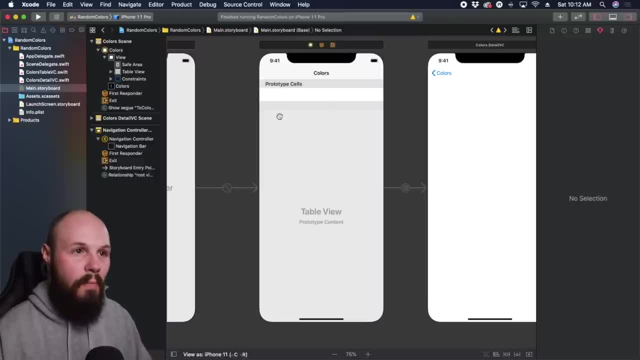 hit prototype cells equal to one. just puts a cell on there. And then now the key thing to remember: with table views- oftentimes people will forget- You need to set the data source and delegate. Let's just let me talk through those. 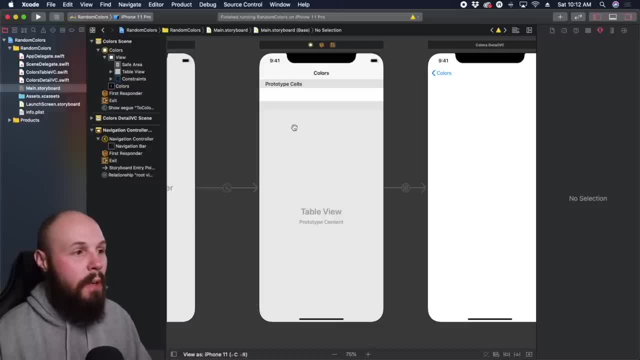 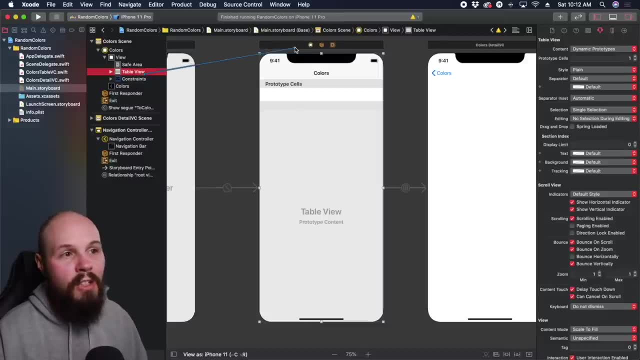 And we'll come back and explain it. So the way to set those delegates here is by clicking on the table view, And I kind of like to do it from here, from the navigation screen here. So control, drag and drag it to the circle. 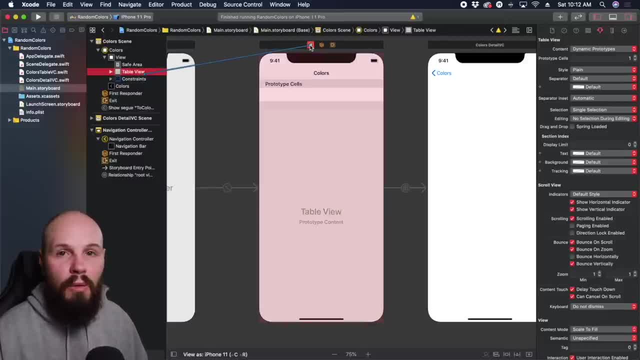 to this view controller. What we're doing here is we're setting the colors table VC as the delegate and data source to this screen, So we're connecting the two. So if you let go of your mouse button here, you're gonna see outlets. 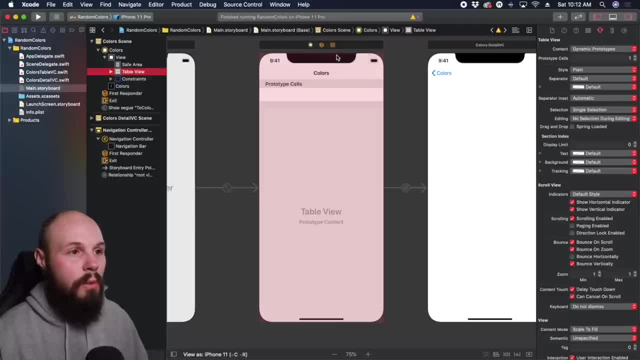 You can do data source and delegate And I believe if you hold shift you can click on bold. maybe not? I know there's a shortcut to this. I don't do this very often, So you can see the dot next to it. 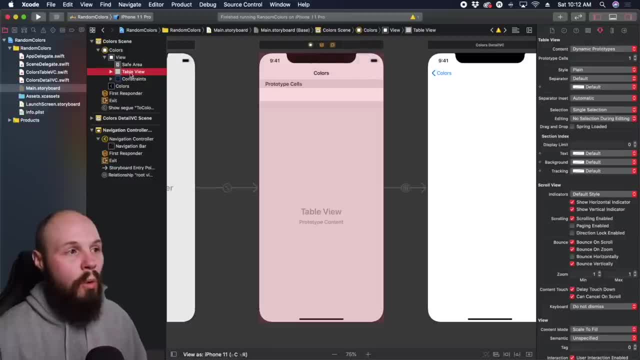 That means we've set our delegate. And now, if you click on data source, let's just hold control drag to double check. Yep, we have our data source and delegate, cool. So if your table view is not working, oftentimes it's because you forgot. 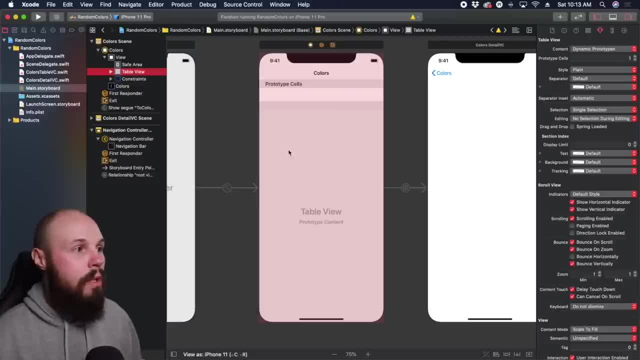 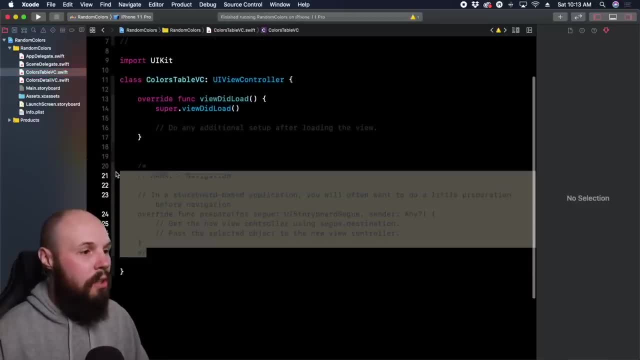 to set your data source and delegate. Let's go back to the table VC code and show you how these two things come into play. So click on the colors table view Now. here let's delete this code. So our colors table view VC has to conform to those now. 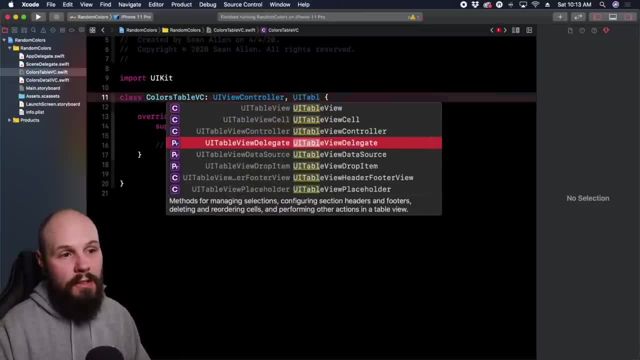 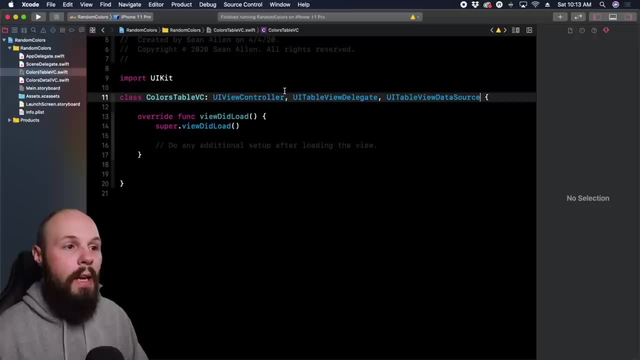 So now you do UI table view delegate, you see there, and then UI table view data source. There it is. So by adhering to these two, now we've connected our table view, but we're getting an error that says it does not conform. 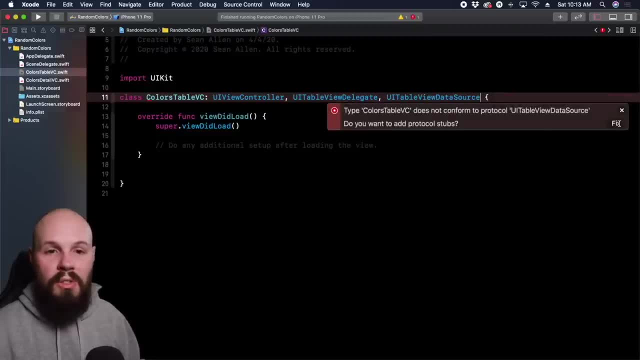 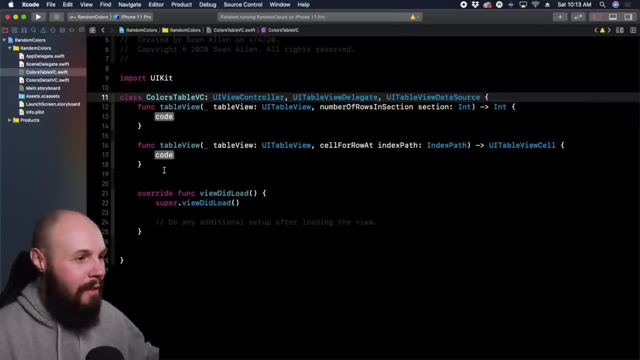 So if you click on these you're gonna see we wanna add the protocol stubs fix. If I'm going too fast, I'm gonna come back and explain this. It's just tough to explain it before I show it. Okay, so that added this to the top. 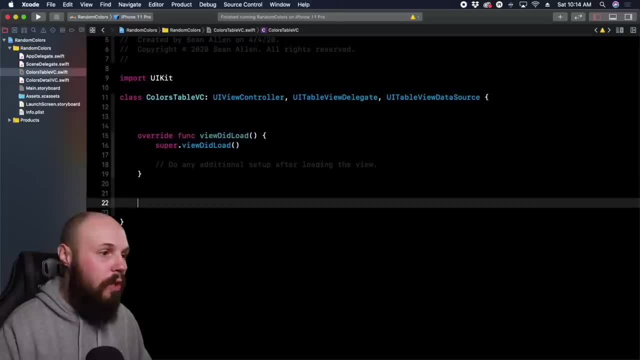 We don't want that in that order. So, command X: you want view to load to be at the top, because that's like the first thing that happens in your view controller And, as a matter of fact, now that you see the structure, 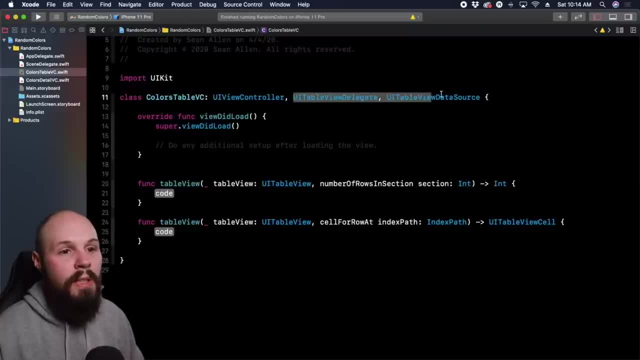 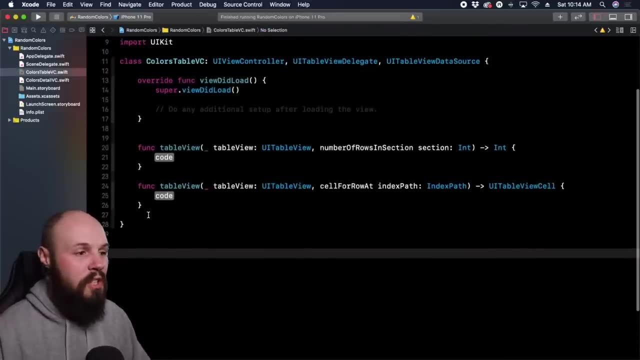 I'm going to introduce what I like to do. So this is like conforming to delegates here at the top. If I'm conforming to a delegate, I like to write an extension on my class, And this is purely for code organization. 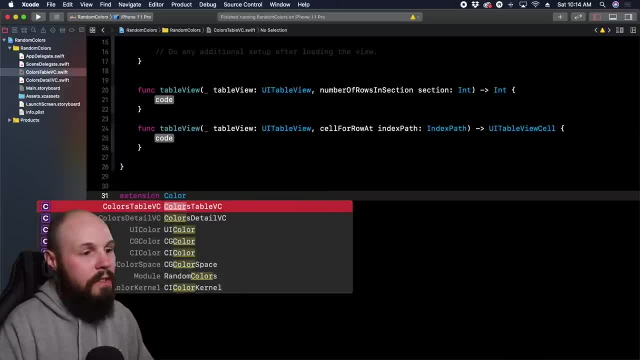 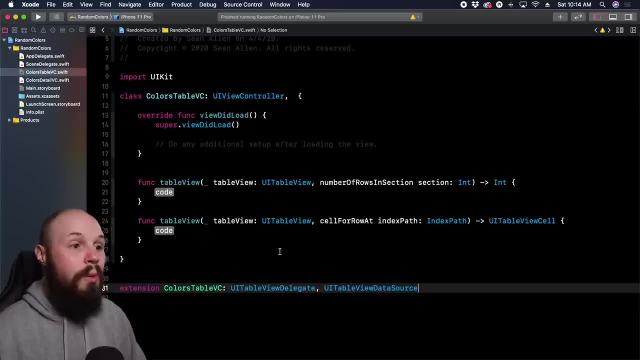 So I like to do extension colors, table VC. And then here I wanna conform to these two, So we'll do command X, command V. We're doing the same thing we just did, We're just organizing it a little more. 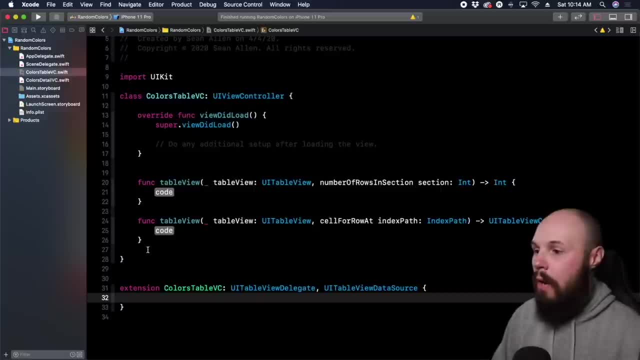 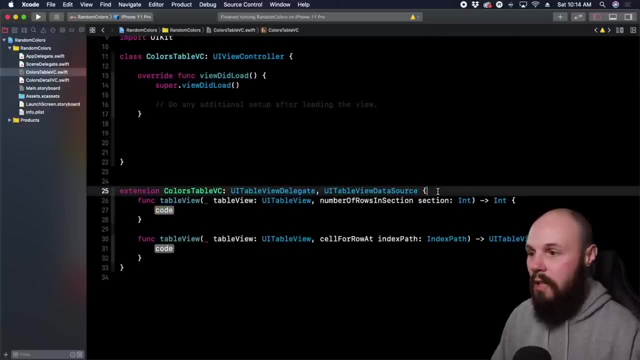 This is all this is. This is code organization. So now I wanna cut these table view functions that we just got and put them in here. So this way you'll see all my normal code for my view controller, which you'll see will play out later in videos. 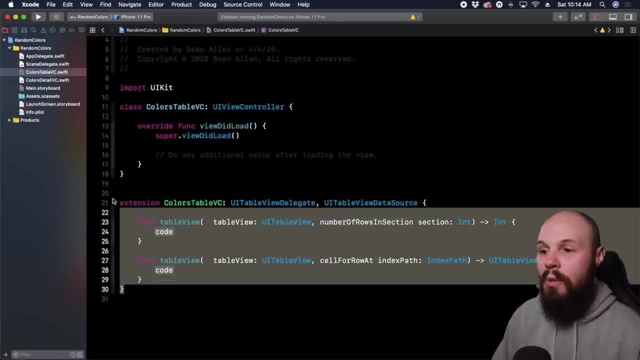 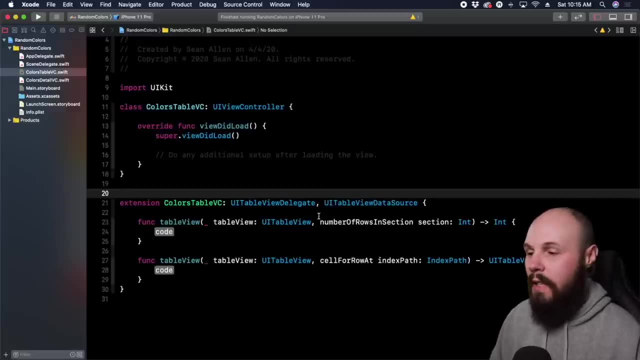 is up here in this view controller. Everything that has to do with the table view is down here in my extension that conforms to the UI. table view: delegate and data source. Okay, so what are the delegate and data source? Let's start with the data source here. 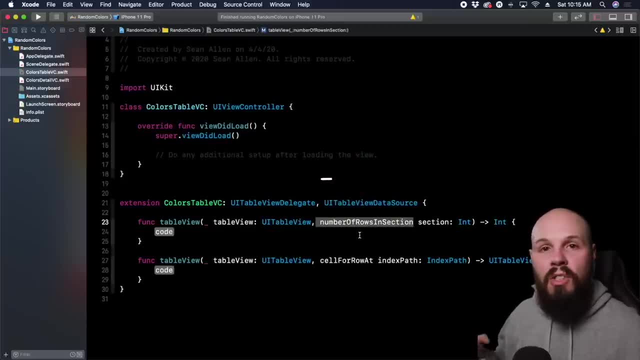 So the number of rows in section Our table view needs to know how many rows to show right. We know it's going to be 50.. So for right now we can return 50.. And the reason I'm returning 50 is you can see here: 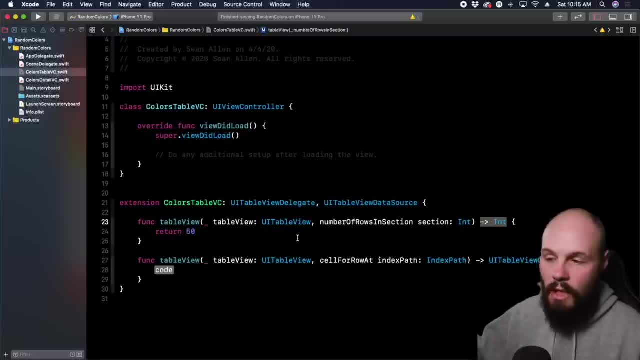 this function returns an int, So I have to tell it how many rows. again an int. So we're going to create a blank table view for now with 50 rows. Eventually, we're going to make this be however many colors are in our array, right? 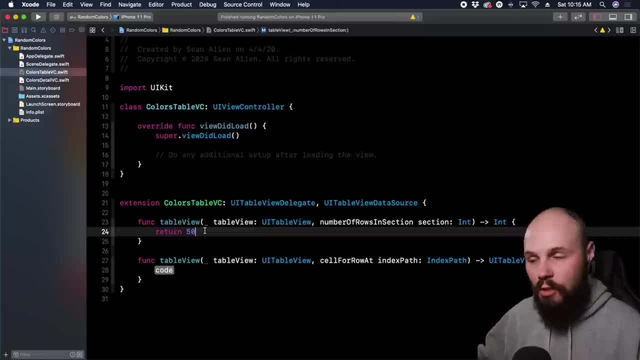 Cause we want it to be dynamic For now. again, just to set up the structure, we're going to put 50.. So that has to do with the data source here. Now this is the delegate self row and index path. 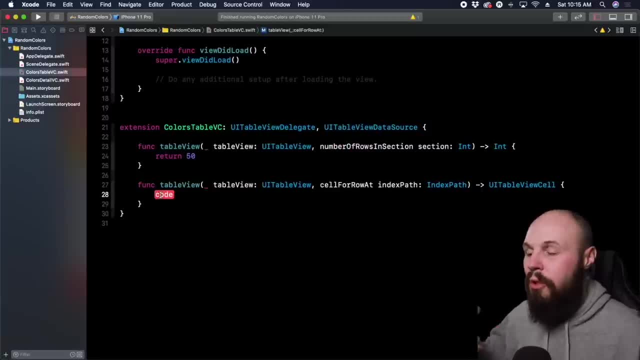 You're going to become very familiar with this function. the more table views you create. This is what's called a delegate method In a simple way. I'm not going to get too deep into delegates. That's a pretty complex topic that a lot of beginner developers struggle with. 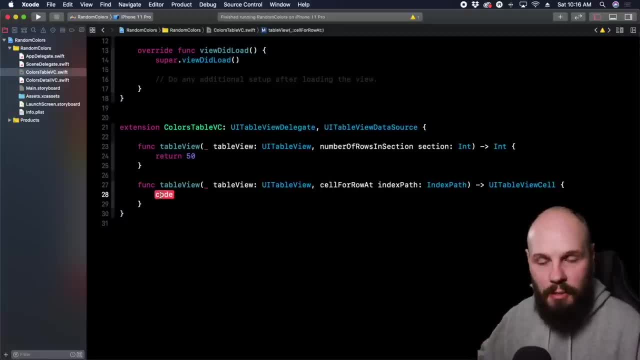 But just to know the concept of a delegate, I think is beneficial. So the concept of a delegate is, to put it really simply, picture this function just sitting back and waiting for something to happen. When that thing happens, this function acts. 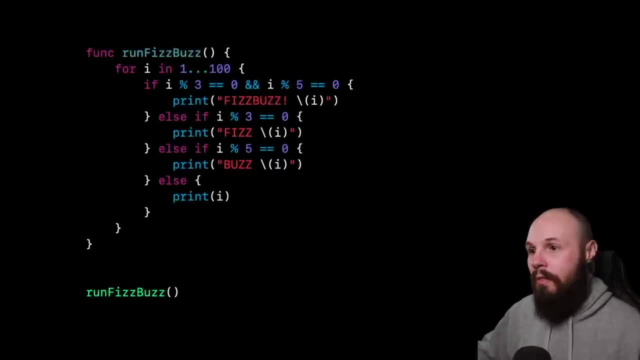 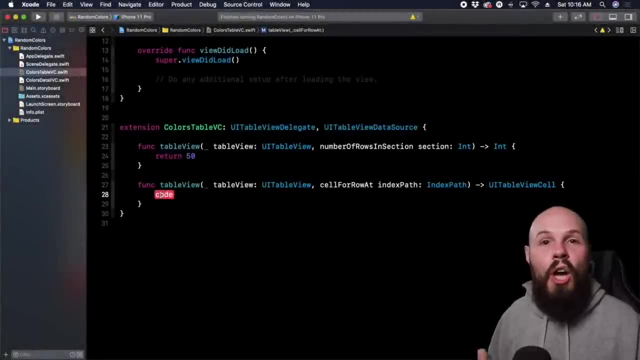 Remember how we used to have to always call our functions? Remember, you know, if I wrote run fizzbuzz, I would have to actually call run fizzbuzz to get that function to run. Well, delegate methods are automatic. You don't have to actually call them to run them. 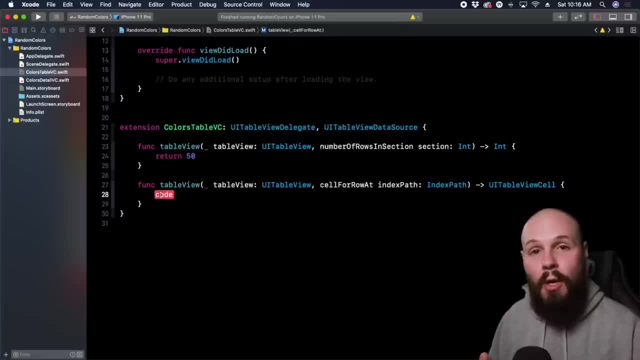 Remember they're waiting for an action And when that action happens they run automatically delegate methods. Again, that's a much deeper topic, trying to give you a big picture overview. But the way this delegate method works is self-row at index path. 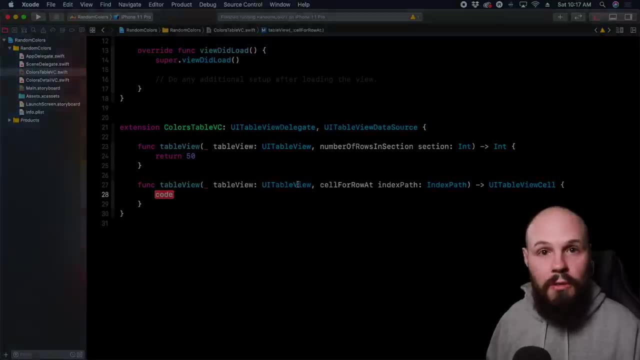 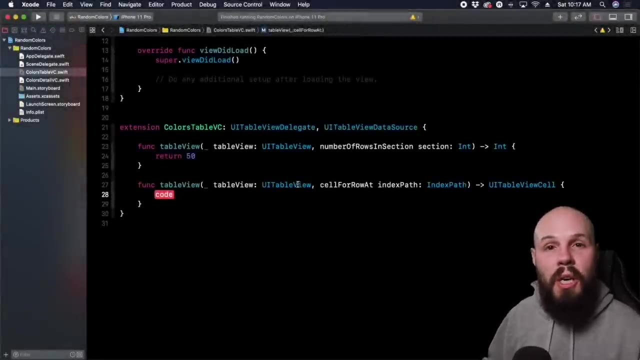 Every time a cell appears on a screen, this function gets called. So imagine you're scrolling through a table view. this function is getting called all the time, right, Because new cells are coming on the screen. So this is where you customize the cells. 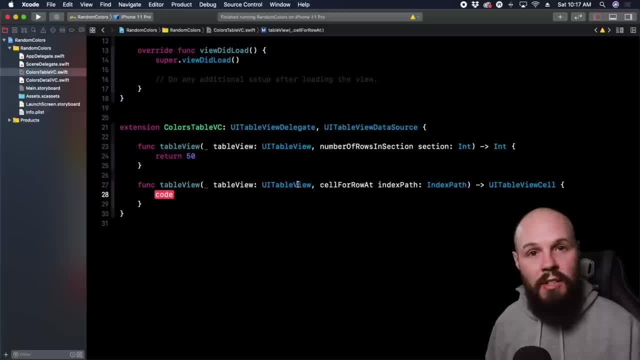 as they come on the screen. We're going to get into that in the logic section of the next video, but I wanted to at least let you know what that does. And again, I'm going to go over that once we have all the code filled in. 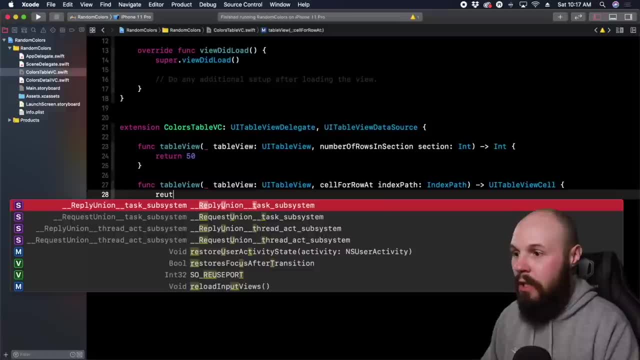 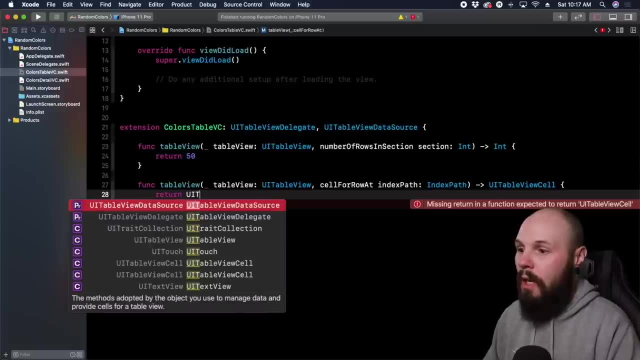 and you can see it in action. But for now we're just going to return and you can see real quick I need to return a UI table view cell. So for now we're just going to return a new empty table view cell, right? 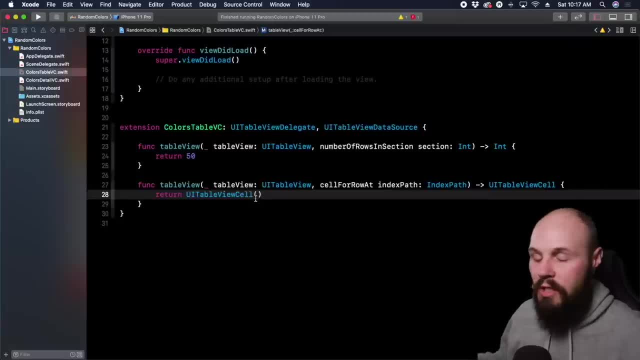 That's what this does. I'm initializing a blank table view cell. Again, we're just setting up the structure In. this function is where we would actually set the color it's supposed to be Again, more on that in a later video. 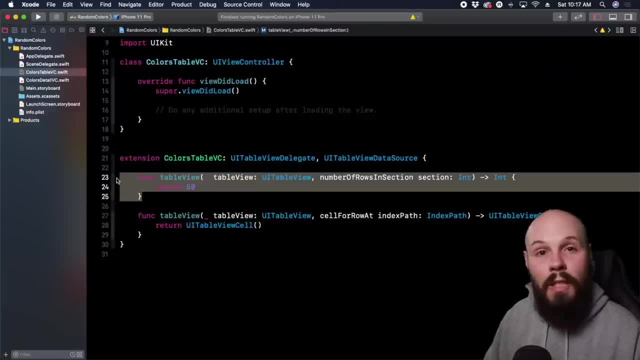 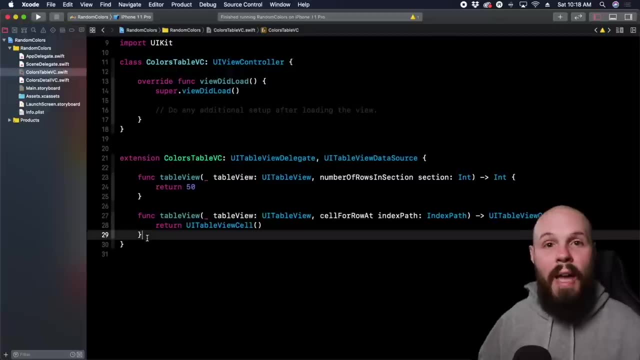 So, again, to review these table view methods: this is what tells me how many numbers of rows I need to show And this tells me what to show in those rows. And, like I said, this delegate method: it just happens automatically. The reason it can happen automatically: 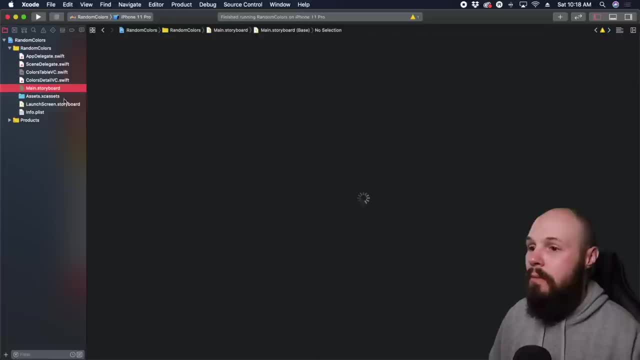 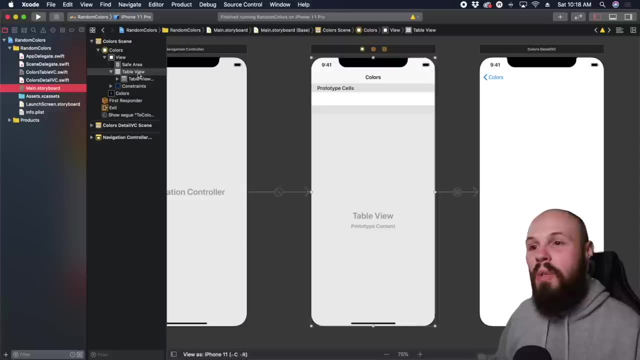 is because, remember back in the storyboard, this is why we set the delegate and data source. Remember how we had to connect the view controller to the table view? Well, this is what's telling the table view what to watch. So that's how that delegate method fires off automatically. 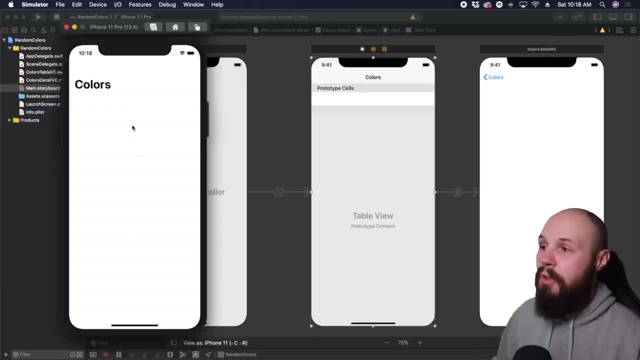 So let's run this and see what we got. So here, as you can see, we have the empty table view, We got our colors, You can see the table view bars And if I slide up, you can see we're scrolling through 50 different rows. 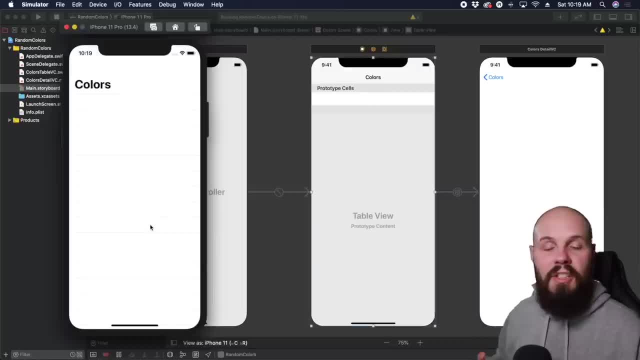 Right now we've got a blank, We've got to fill it in with colors, but this is just setting up the general structure of our table view. And now actually, let's go back. And because right now, when we tap on a cell, 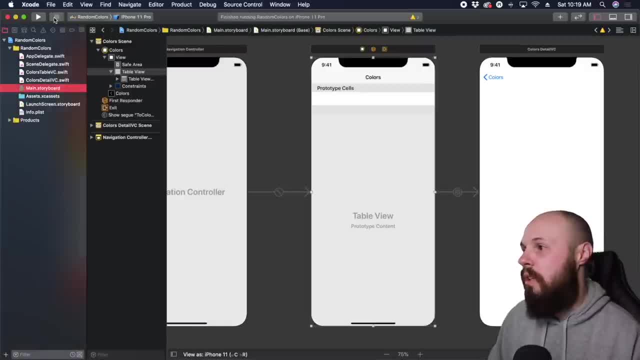 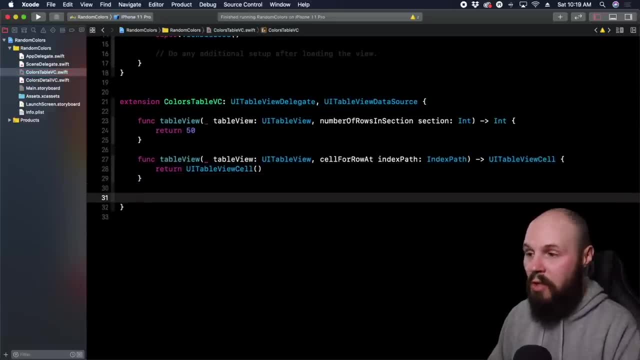 nothing happens. right, We're selecting it, but nothing happens. So let's close this and let's go back to our colors table VC. And again, another delegate method that we can implement is, if you just start typing did select, you'll see did select row at index path. 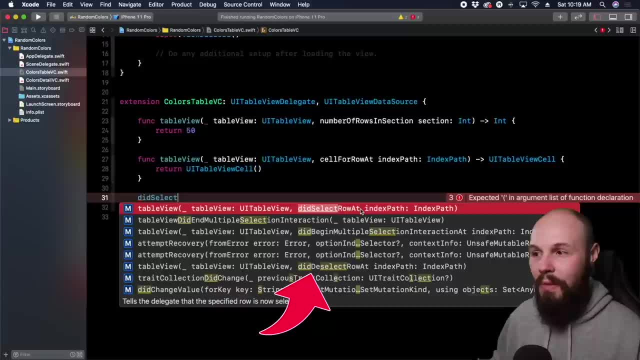 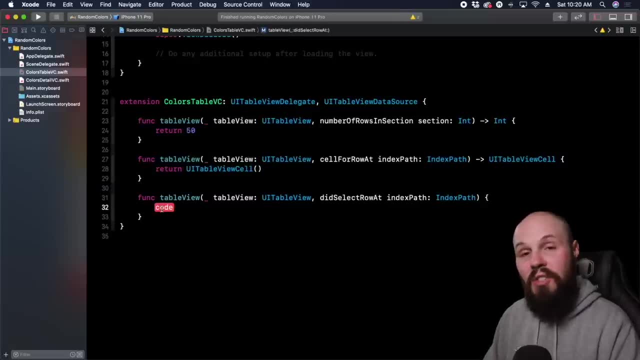 Be careful. There is a one that's called did deselect. Don't want that. That's another error that a lot of people make sometimes. So did select row at index path, And now here's we want to again, just like we did with our button. 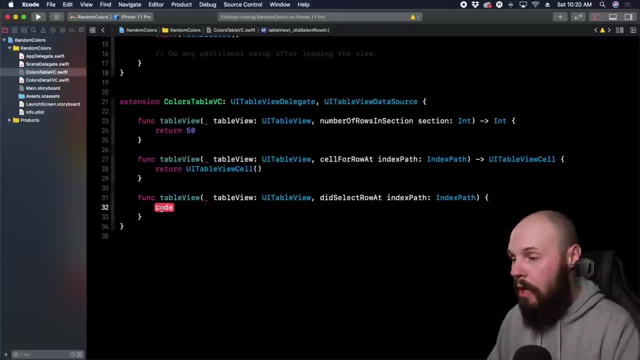 Remember I said we were going to replace that button with when you actually tapped on the row. We're going to do perform segue with identifier. It was to detail, to color. I'm living dangerously right now And I'm kind of hoping it crashes. 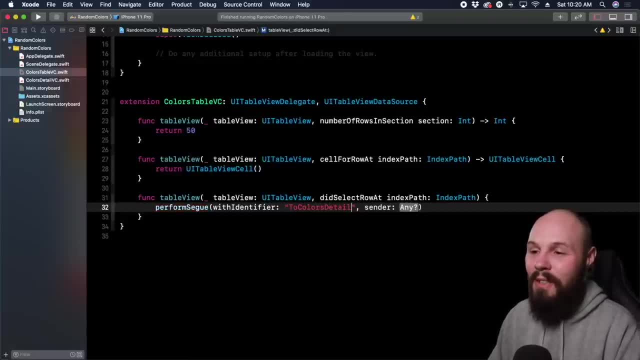 I'm going from memory on what we named this to colors detail VC. I hope that's right, But if I'm wrong it's going to crash And this is the danger of kind of like using the string And why I always went back. 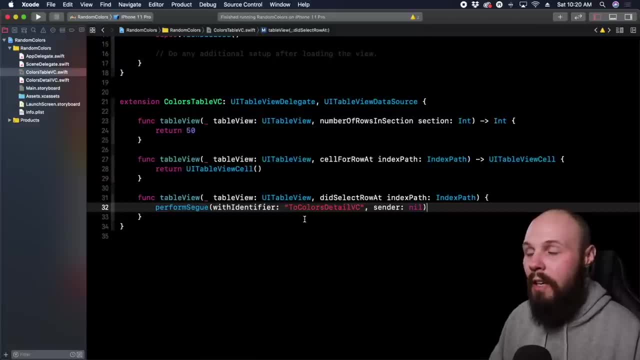 and copied and pasted in the name of the segue that we were firing off. So again, when we tap on a row, we're going to fire off that. two details: VC. So now let's run it and see if we got our navigation working. 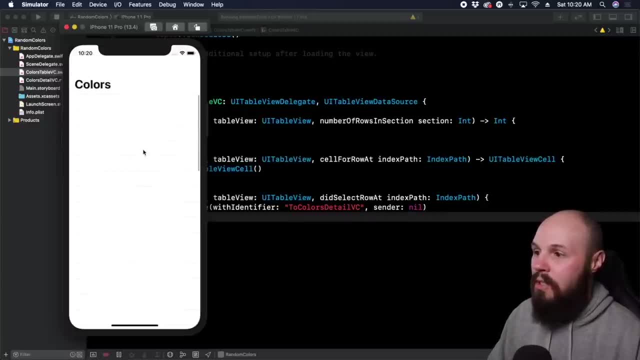 So again, here's all of our cells. right, I'm scrolling up and down. Let me tap on a cell. Nope, didn't crash. That means I got the name right, And you see, now we pushed the detail VC onto the stack. 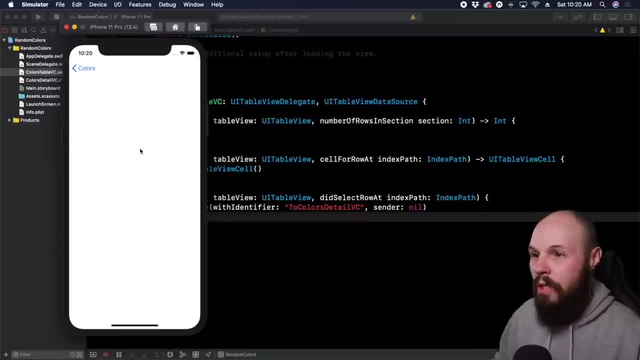 And eventually this is going to be whatever color we selected. But again, we're just building the basic foundation in the navigation of our app. So again we got the basic structure of our table view down. Tap on a row, There you go. 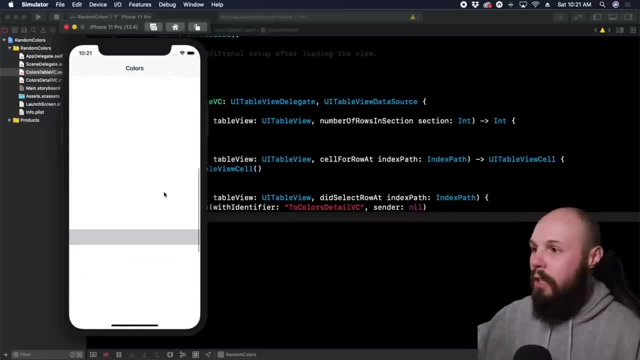 Now we just need to fill in the logic on generating random colors to fill each cell And then when we tap on that cell, we want to pass whatever color we tapped over to this view controller so it knows what color to set its background color to. 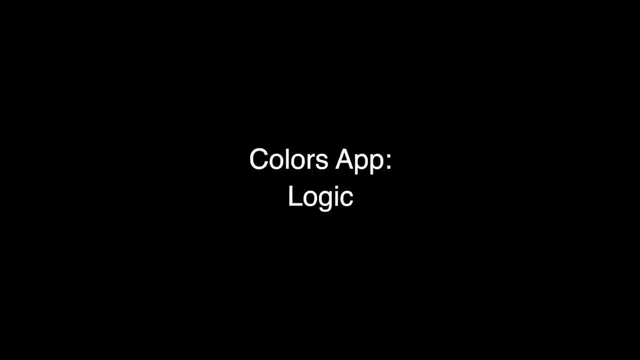 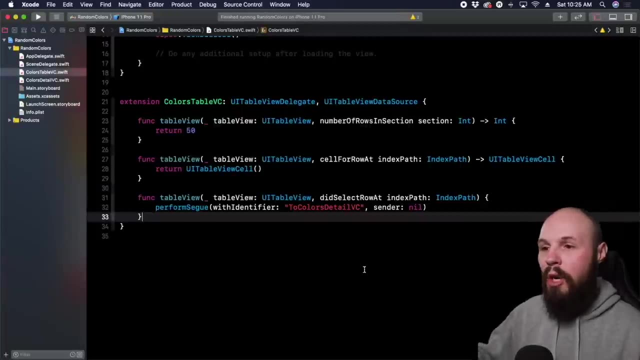 All right, Let's move on. In this video, we're going to start writing all the logic to populate the random colors In our table view And again my project has left off exactly where the last video left off, so you didn't miss anything. 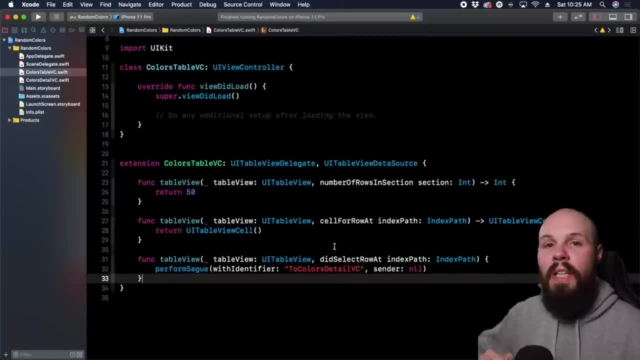 Here we are in the colors table VC, So let's think about what we need. We're going to need 50 random colors. That's what we got to populate it with. Now, table views always take an array, So remember, an array is a list of items. 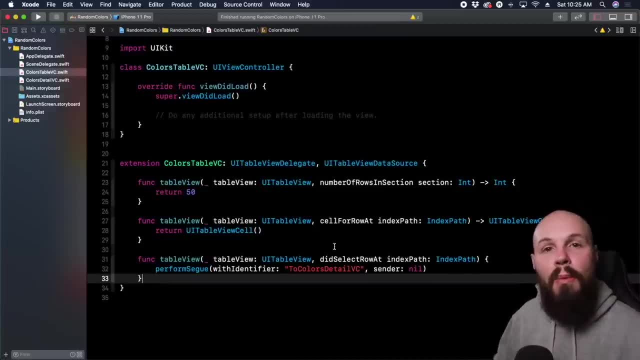 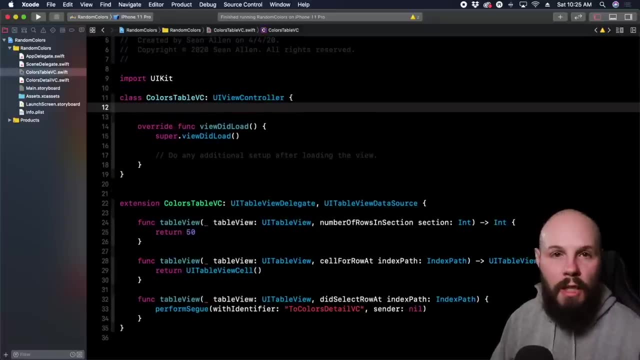 So we're going to need an array of random colors And our table view is going to populate based on that array. So let's create that array first And just keep that in mind. Table views And collection views: They need an array of something to show. 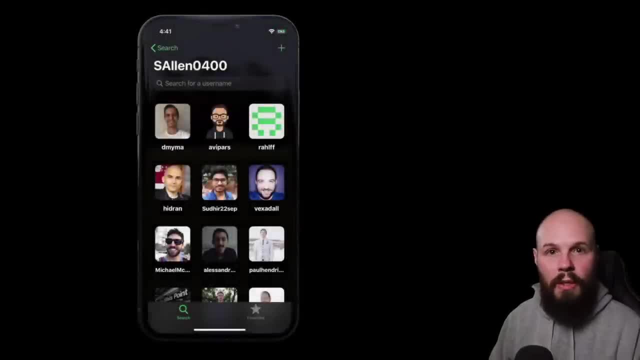 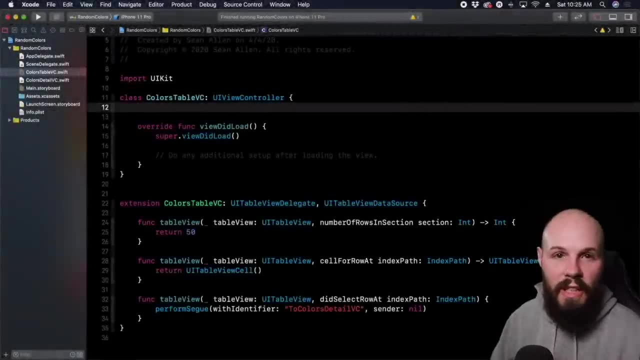 For example, here on the screen you see a list of my followers on GitHub. Well, in order to populate that collection view, I need an array of followers. So that's why table views and collection views are always going to need an array. 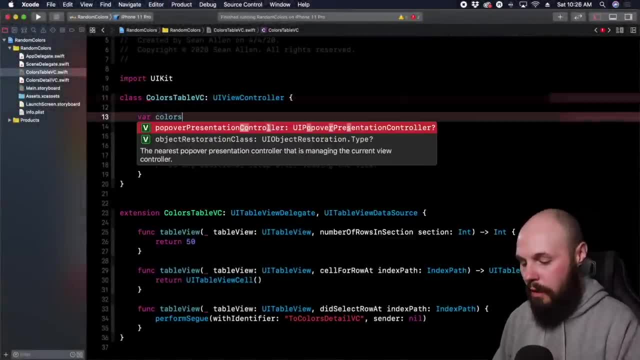 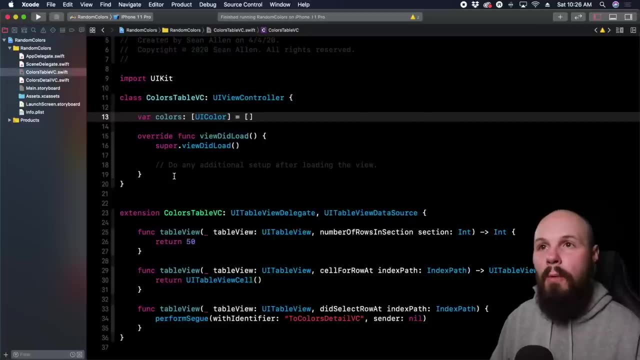 So let's create that array, So var colors, And that's going to be an array of UI color And that's going to equal, right now, an empty array. So to populate that array we need to create 50 random colors. So to do that we need a for loop. 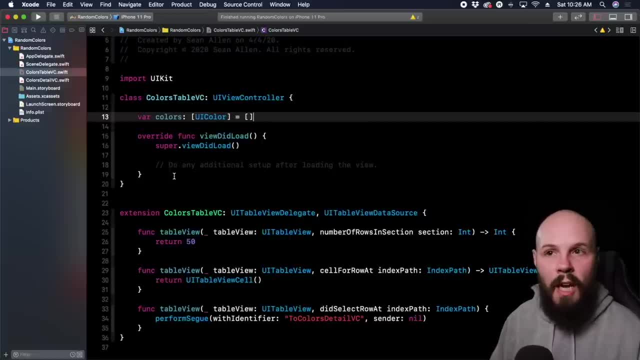 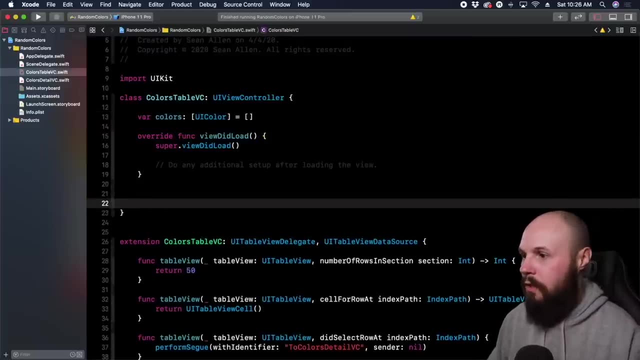 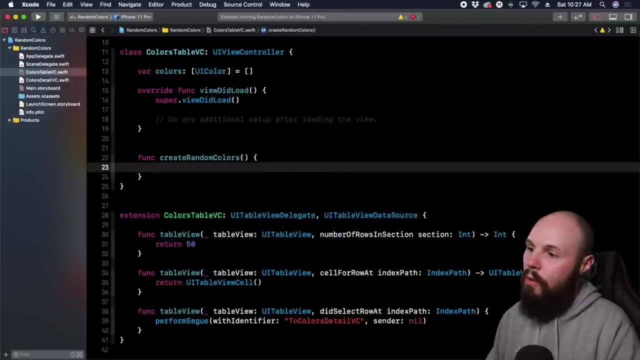 That iterates 50 times, creating a different random color each time and then appending that color to our colors array. OK, So let's do that here. Let's create a function, Func, create random colors And close. So for i in 0 dot, dot up in 250.. 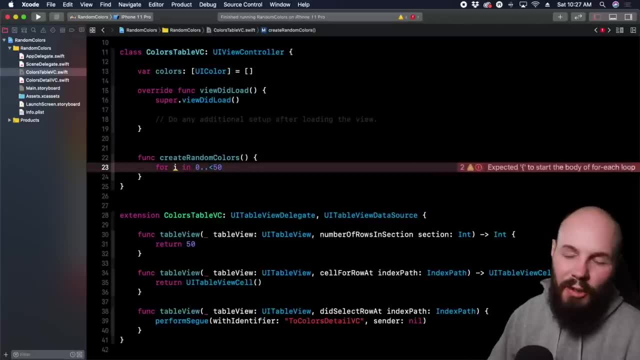 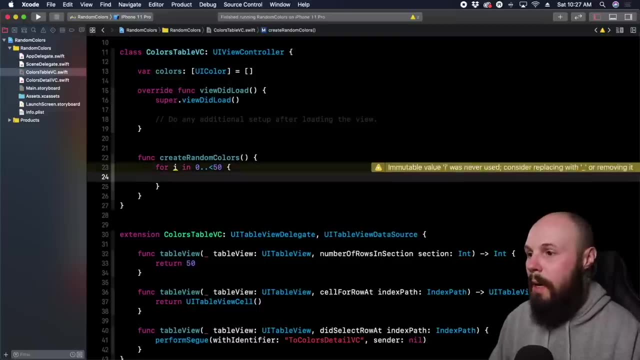 Because, remember, if I did 0, 250, that would give me 51. So up to, but not including, 50 is what that less than sign means for the ranges. So this is going to count 50 times And again, we're not going to be using the i so we can do the underscore. 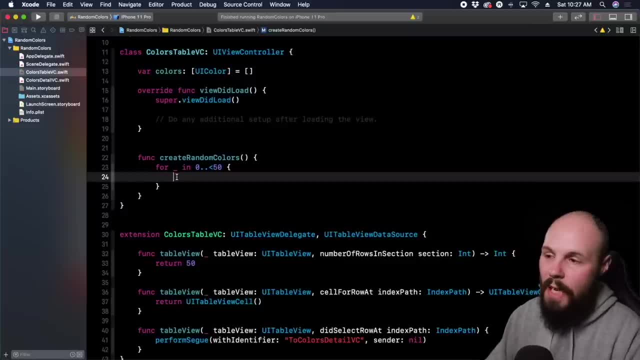 It just takes the i out of it, basically meaning we're not going to use the name of the variable. So here we want to create a random color. OK, how would we create random colors? Well, rather than writing that here in our for loop, 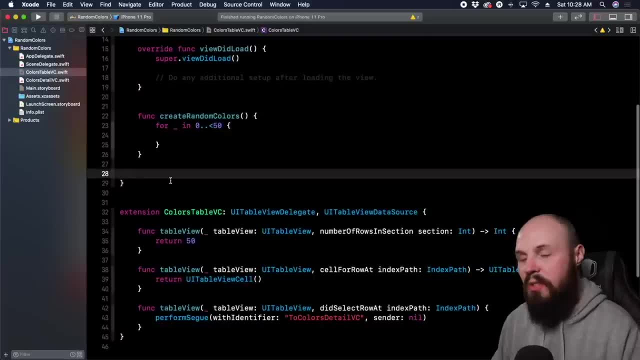 let's actually break it out again, Again, to keep the code nice and compartmentalized and also to help you learn, because you can see how all the chunks of code come together. So I'm actually only going to do one space in between. 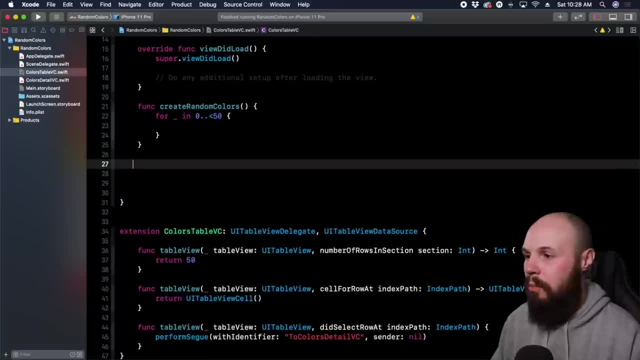 Normally I do two spaces, But because my screen is so blown up that takes up a lot of space. So let's do func, create random color, And we want this to return a UI color right, Because, again, this is kind of like a little factory. 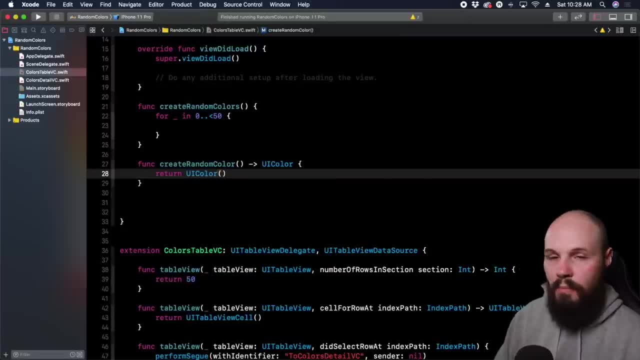 So real quick, return UI color. That's just a blank one, That's temporary, so Xcode doesn't yell at me within there. But this is going to be like a factory that we're going to run it and it's going to spit out a random color. 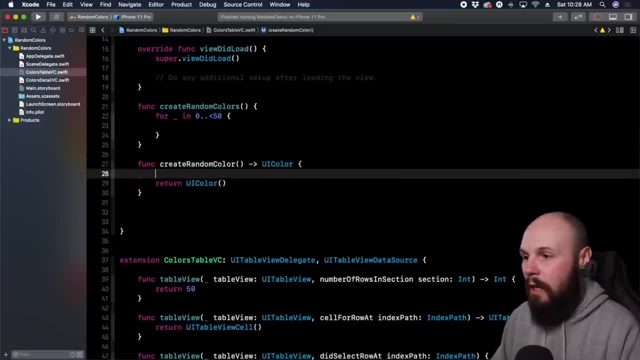 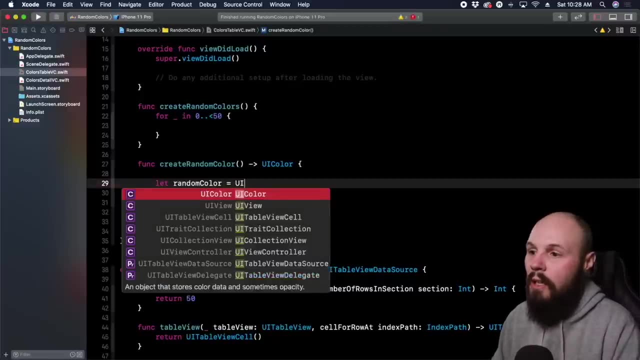 And again that's why we're spitting out UI color. So here let's say, Say let random color equals, And here's how you initialize a UI color. So UI color, And you can see we can do there's. 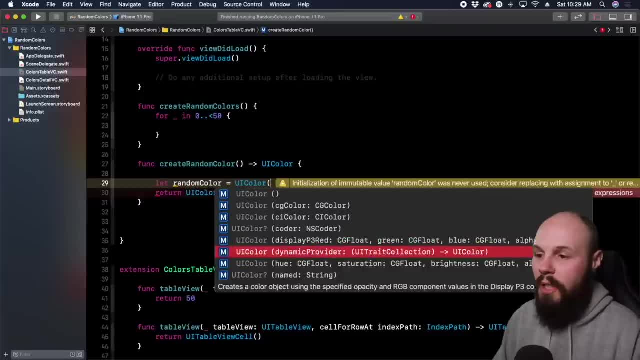 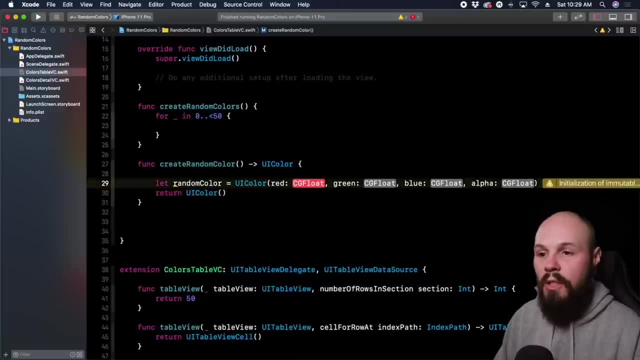 many different ways to do it with hue display p3, named, I like to do the red RGB basically. So we need a red value, which is a CG float, green, And the CG float is a value from 0 to 1, right? 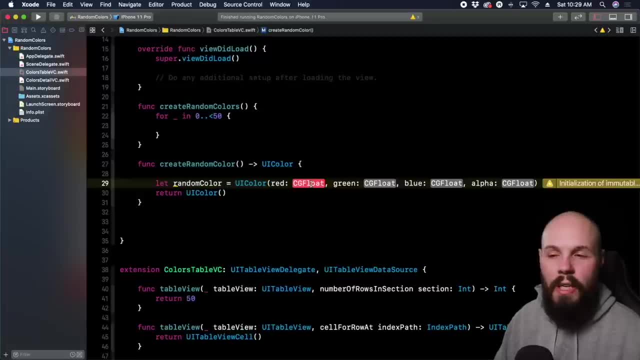 All 0s is black. I believe All 1s are white. Yeah, I think I got that right, But we want a random color. So what we want is a random float from 0 to 1.0, right. 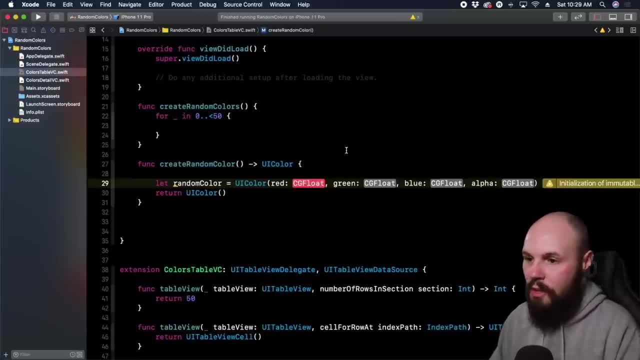 It could be 0.76, right, And they combine those numbers. So what I can do is CG float, And we've done this with the N right Dot random, And we want a range of 0 up to 1.0.. 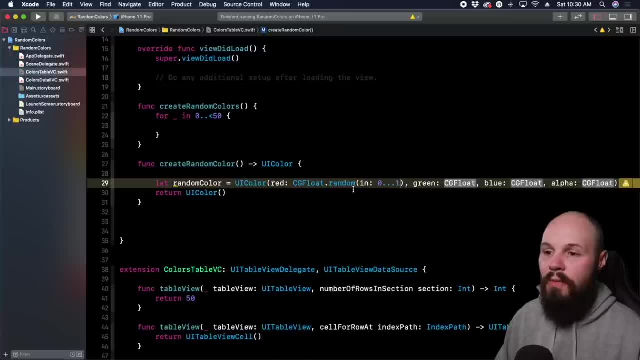 We want to include 1.0, or just 1.. So that is going to give us a random float for the red, And let's actually put this. You can do this with functions, by the way. You can separate them by parameters. 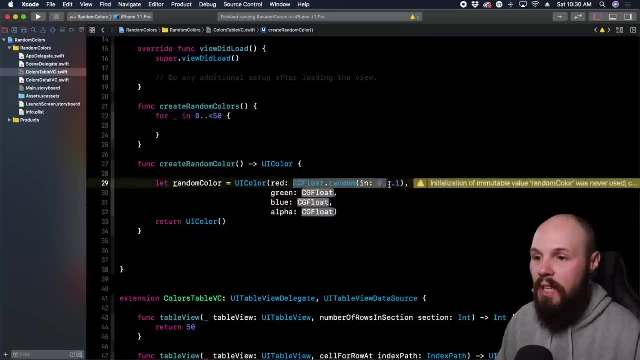 So it lists them out. So that was a pretty long one. So now let's actually do this multiple times here. This is going to give us a alpha is opacity. So if you have alpha of 0, you're not going to be able to see it. 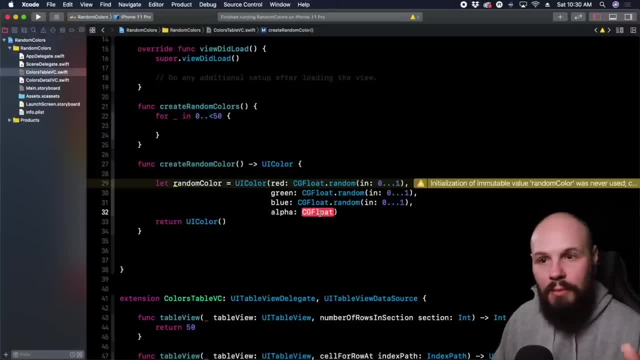 If you have alpha of 0.5, it's going to be like faded out. You're going to be able to see through it halfway. Or 1 is full opacity, We want 1.. So here we're creating a random color, right? 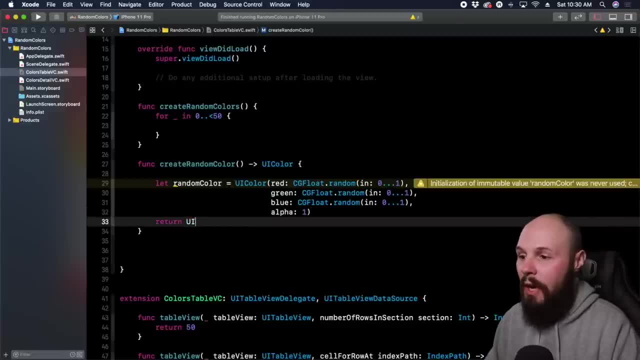 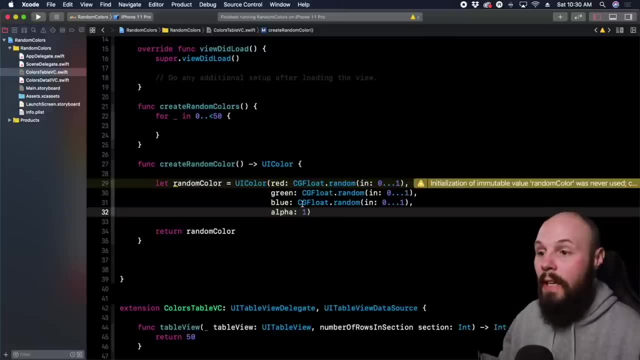 CG float dot random, And then now we want to return that random color, Random color. And again, if you have any questions about this function, feel free to leave a comment in the Slack Again. we just needed a value for red, green and blue. 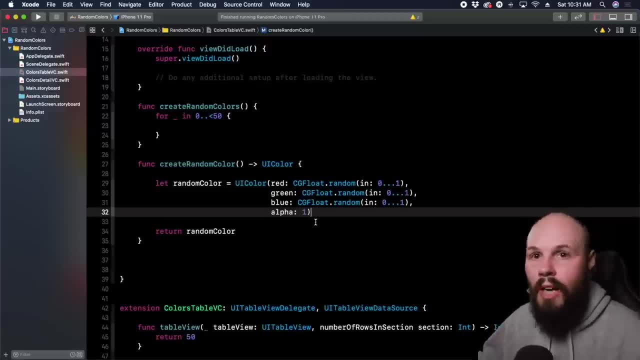 And that value has to be from 0 to 1.. So again, 0.25,, 0.48, right? So we're just creating a random value from 0 to 1.. So it could be anything random, And then we're going to combine those to get our random color. 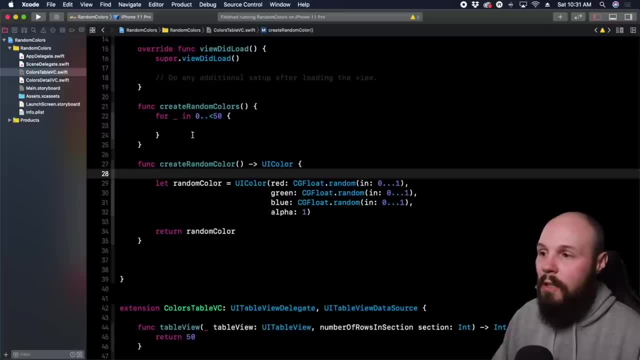 So this create random color function is what spits out that random color. So now what I can do is up here in our for loop I can do colors dot append right, Because we want to add a new color every time. this for loop. 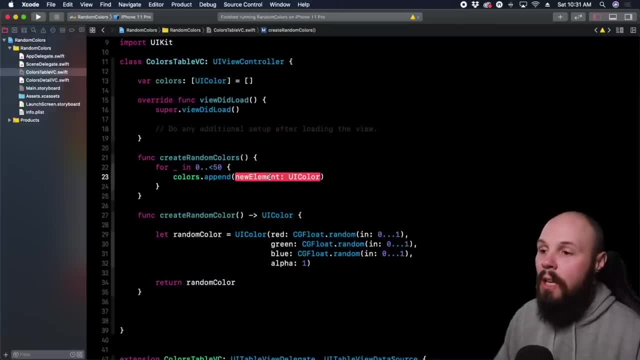 goes, And we're adding it to this colors array up here on 13.. So we need to pass in a UI color. You can see that's what I need to pass in Well, here. this create random color function spits out a UI color, returns one. 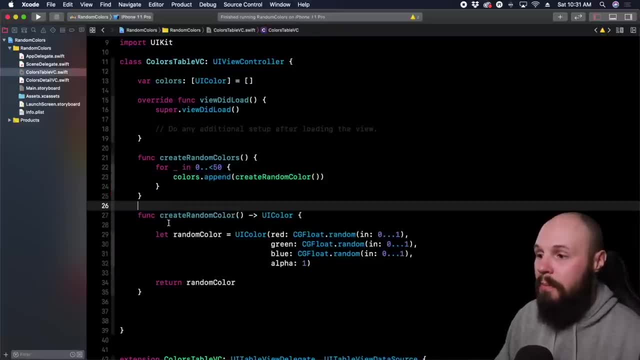 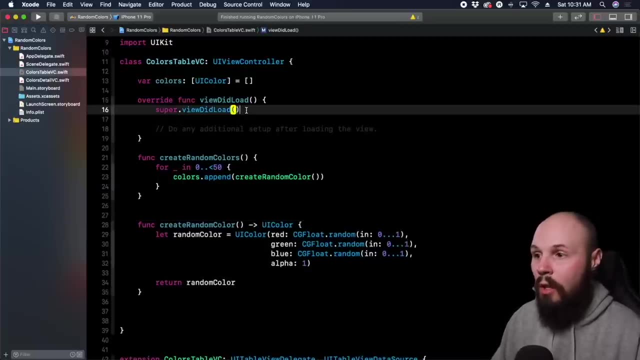 So I can do create random color in this function up here, Tighten this up a little bit. So here, what this function does, called create random colors, was actually- let's call it before I forget- create random colors. That happens in view to load. 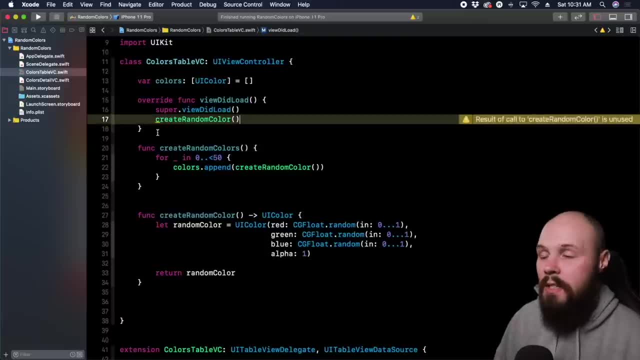 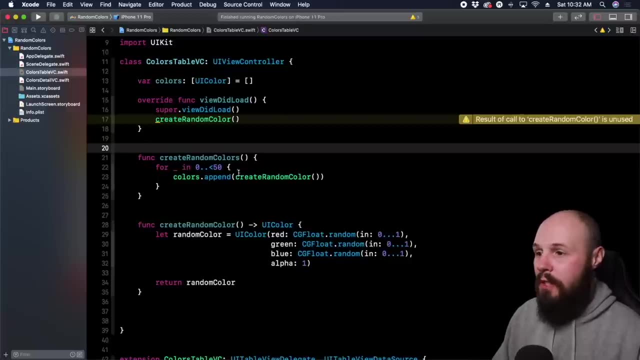 So view to load happens as soon as the screen is loaded into memory, So it's one of the first thing that happens in your view controller. Oh man, I named these poorly. Good example of how naming is important, right? See how this is. create random color. 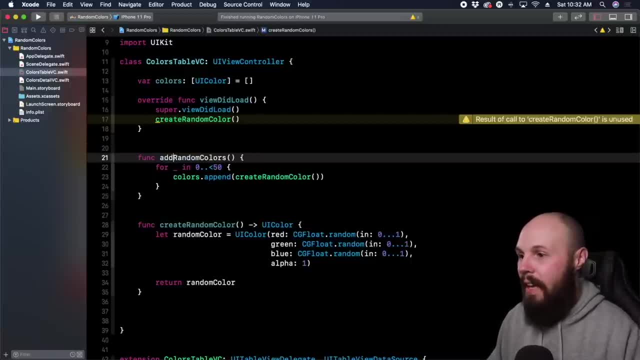 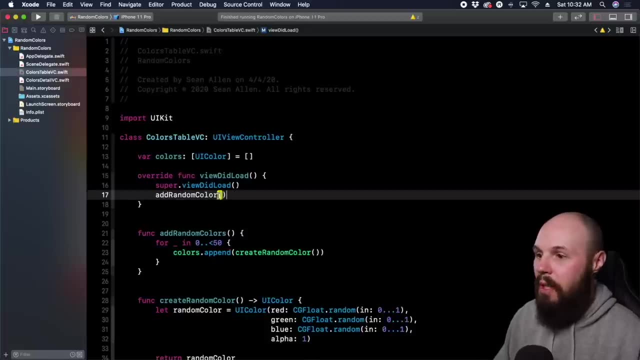 this is create random colors. Let's say, let's call this: add random colors, just to really differentiate them, Because, see, I put in the wrong function there. That's what happened there. So, in view to load, we're adding random colors. 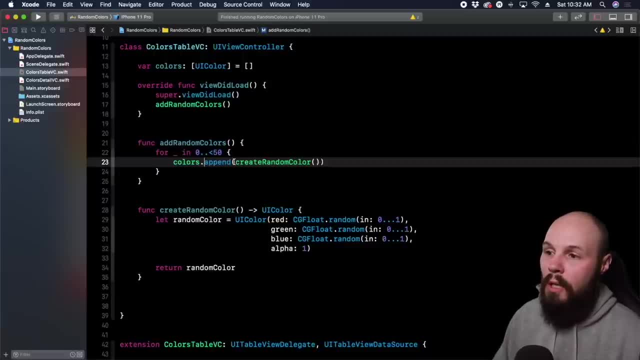 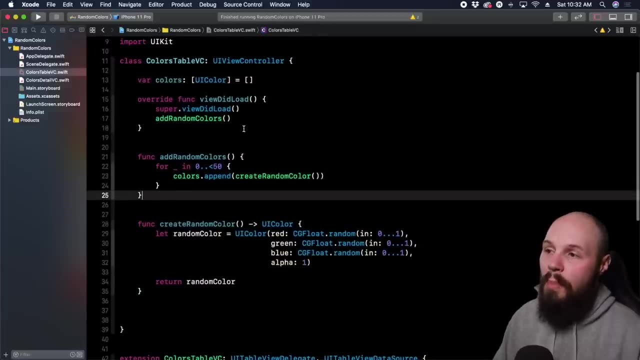 So that's what's happening here, And then, every time this for loop goes, we're going to call create random color, which is going to fire this off, which is going to generate the random colors. So, in view to load, what happens is our colors array. 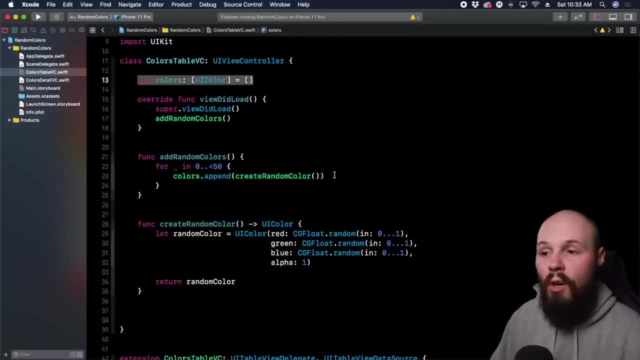 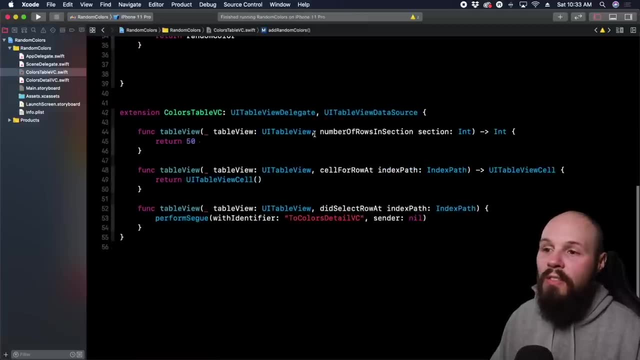 gets filled with 50 random colors. So now that we have our array, we can use that in our table view right. So down here in our table view methods, remember we put them in the extension instead of returning 50 for number of rows and section. 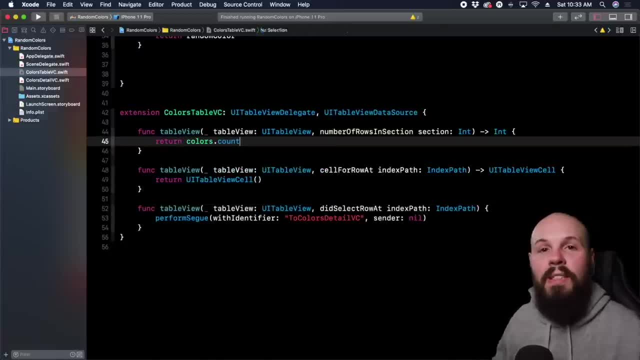 we can return colorscount. Remember, we wanted to make this dynamic. However many colors are in our color array, that's how many rows we want. So instead of passing in a hard number of 50, colorscount, that number is going to be 50, again. 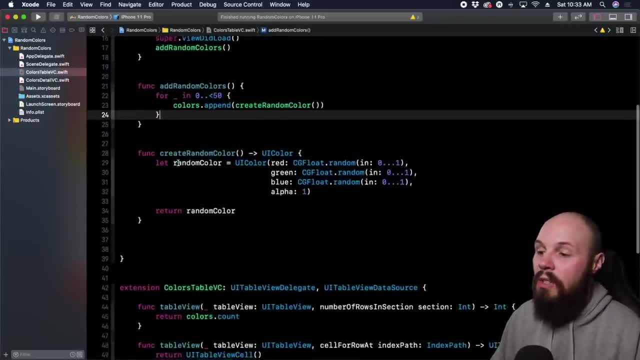 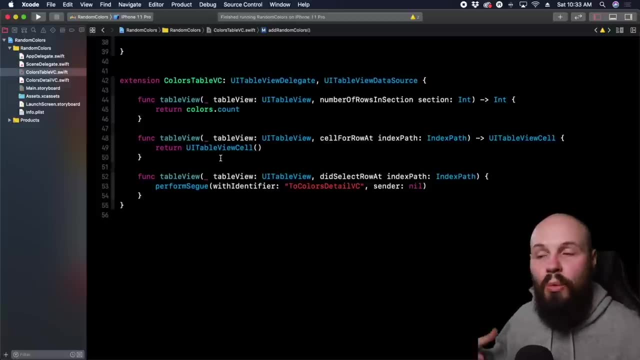 because we're appending 50 colors into that. So now remember, the table view needs to know how many rows I need to show and what I need to show in each row. So in order to tell it what to show, we need to write some code here in our cell for row. 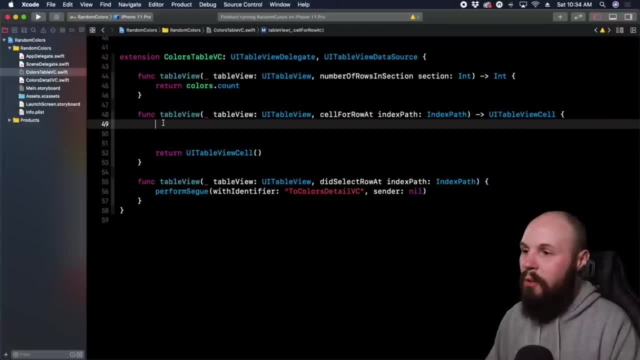 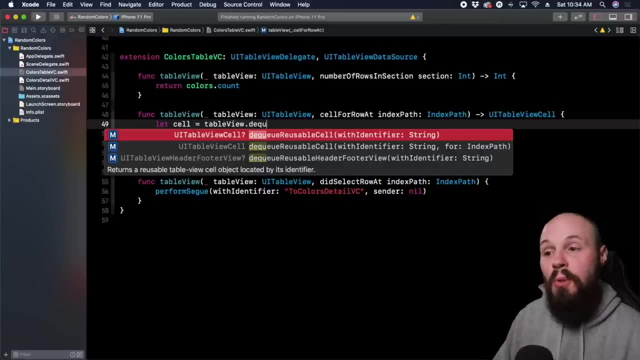 at index path method. So to do that we need to get access to a variable called cell. So we're going to create that. let cell equal table viewdq. we see reusable cell with identifier. So our cell has to have an identifier here. 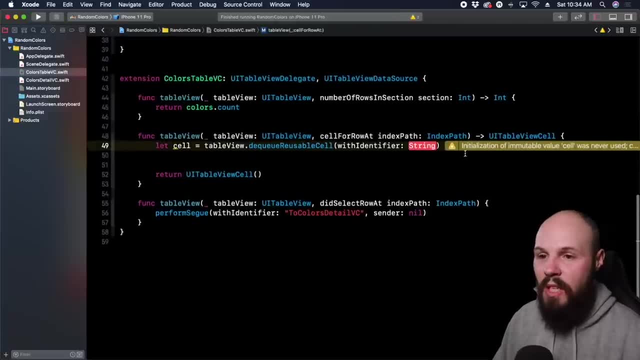 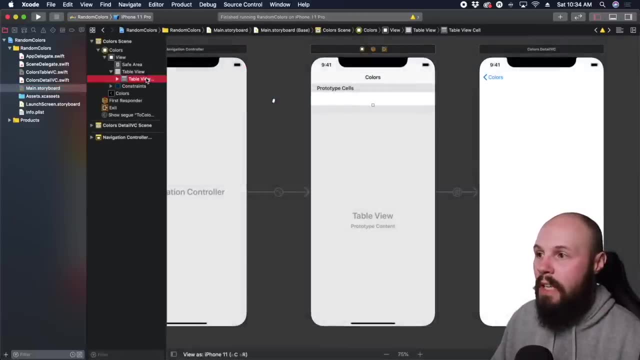 just like our segue. I'll come back and explain this function in a second once I get this string. So again in our mainstoryboard, click on your cell here, your prototype cell that we added. table view cell here in the right pane. 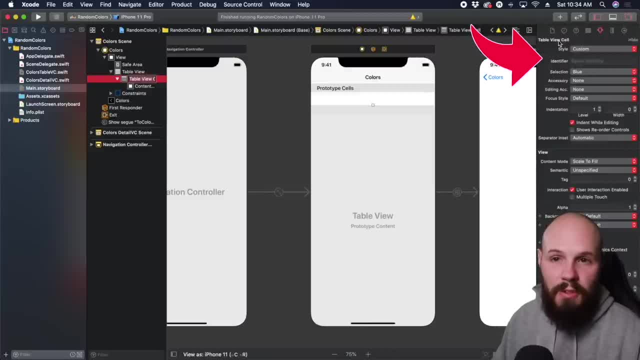 we're going to have the identity inspector- I'm sorry, the attributes inspector. And you see, the table view cell. we have an identifier. This is the reuse identifier. again, we'll talk more on that in a second. So we just want to name this color cell. 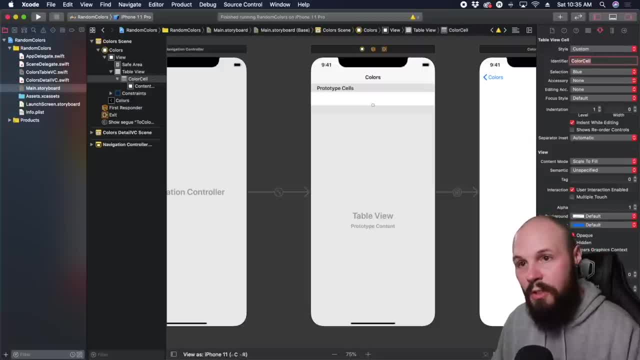 Keep it simple again. I'm going to copy and paste that: Make sure you hit return. that's what actually makes it go, Trust me, so many times I've forgotten to hit return and things weren't working. Silly little error, but it happens. 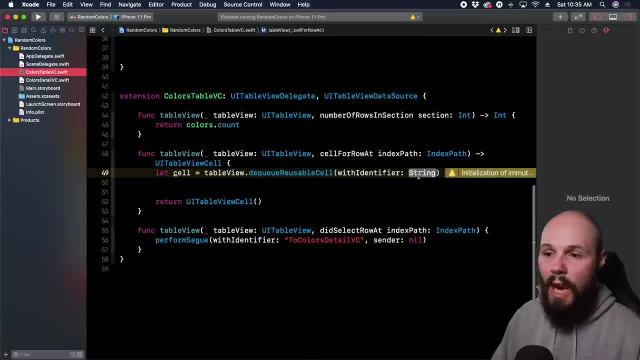 And go back to our code here in the colors table VC. So now I'm going to paste in that string that I just copied: color cell. So now we have this variable called cell, which is our dq reusable cell with the identifier of colored. 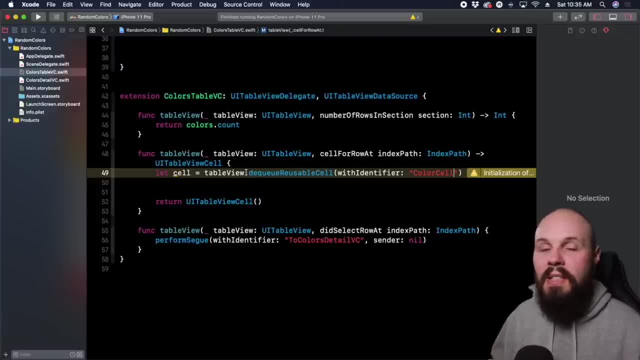 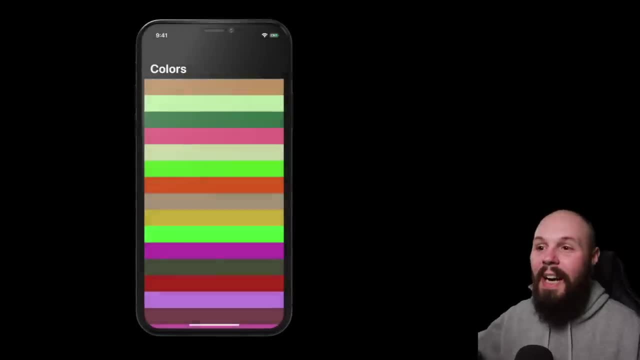 So what cell reuse means is basically the table view controller. Remember, we have 50 rows. Let's- actually I'm not going to run it yet, my code's broke, but I'll put up a picture on the screen. This table view has 50 rows. 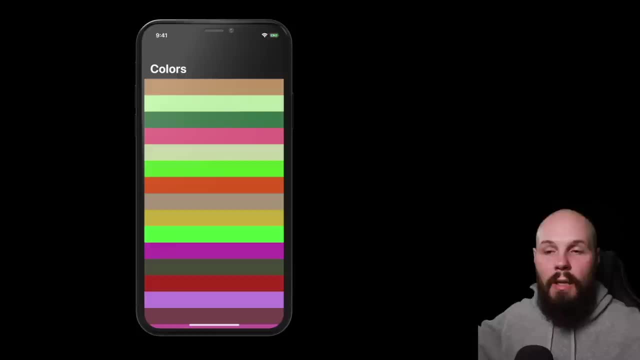 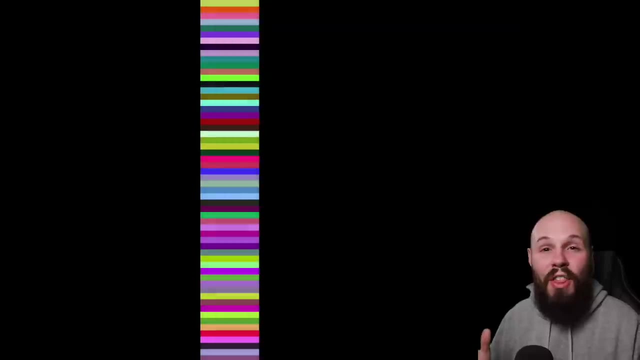 However, it's not for all 50 rows that are populated. The iPhone is smart enough to only use what's visible. Imagine if you had a table view of 1,000 random colors. Well, that's not all going to get populated right away. 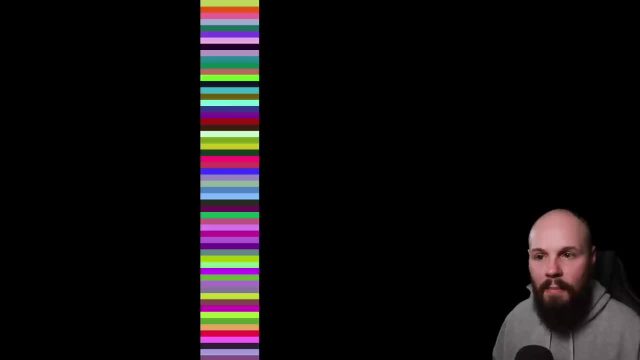 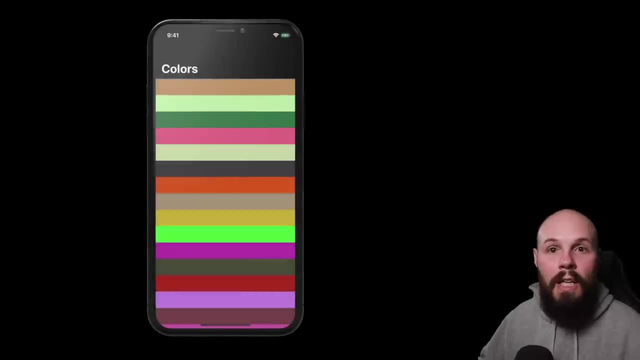 That would be poor memory usage, that you would get poor performance out of that. So what the iPhone does is it only uses what's being shown. So, as you're scrolling down, as soon as this cell falls off the screen, it gets rid of its data. 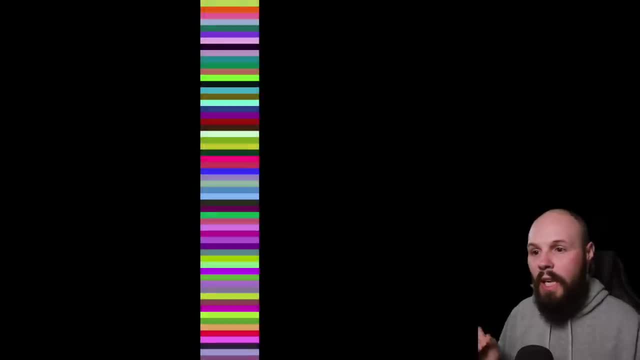 and is ready to be reused for the new cell that comes on the screen. So again, if you had 1,000 rows of cells only, whatever, like 12 to 15, I'm just saying what is visible on the screen. 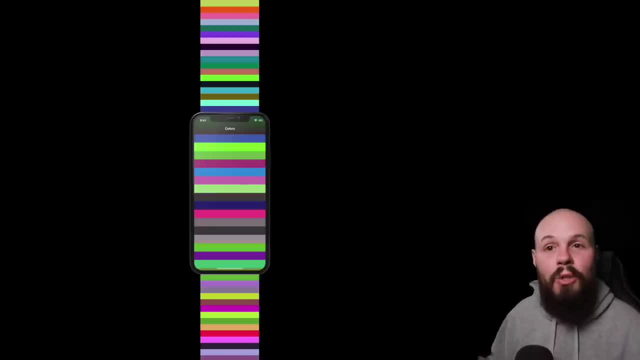 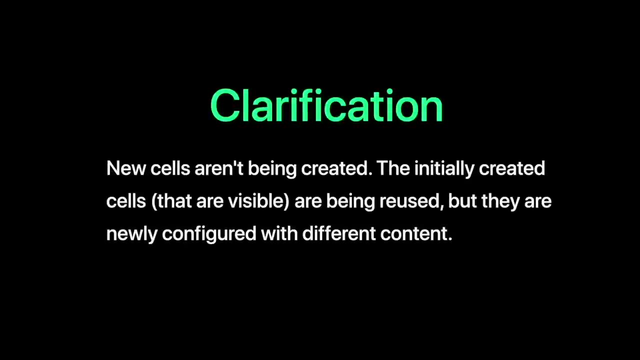 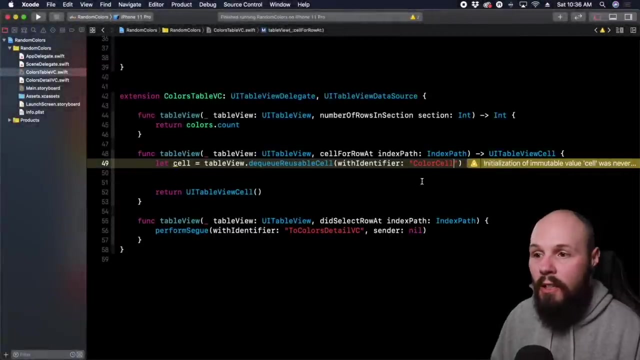 are cells that are actually being created. So new cells are constantly being created as you're scrolling up and down. That's why this self-wrote index path function that we're looking at here fires off all the time. So that is what is a reusable cell. 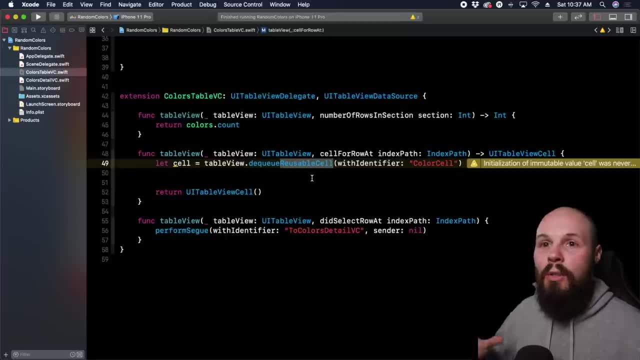 That is a little bit more of an advanced topic. I just kind of gave a little overview. I mean it's not super advanced, Developers should know that. But again, this course is like your very first exposure to this world. It might be a little advanced for that. 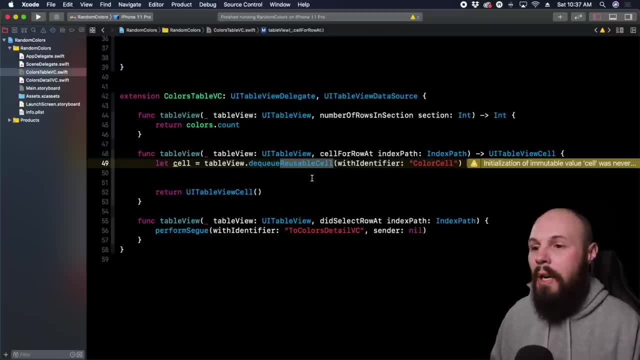 But, yeah, you may have to do a little bit more work on that. But again, this course is like your very first exposure to this world. It might be a little advanced for that, But, yeah, you may have to do a little bit more work on that. 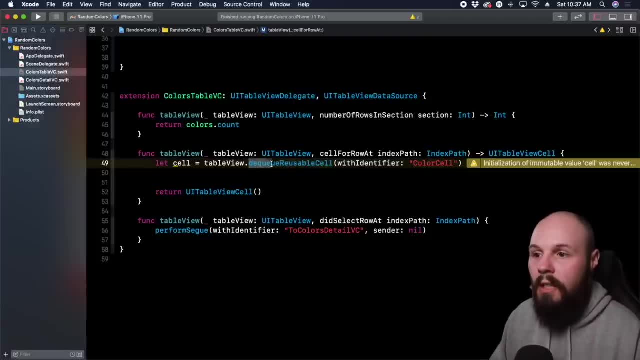 But again, this course is like your very first exposure to this world. But again, this course is like your very first exposure to this world And we're going to do a little bit more research on reusable cells. But that's what we're doing here is we're getting that reusable cell. 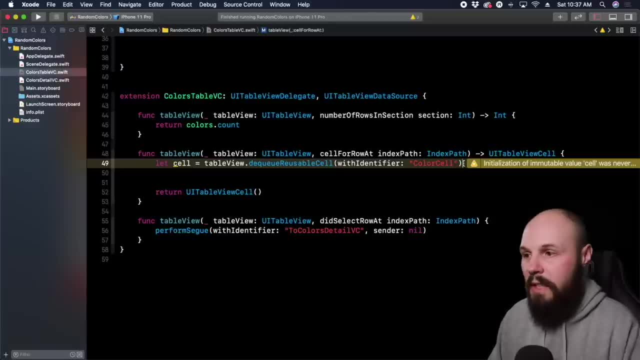 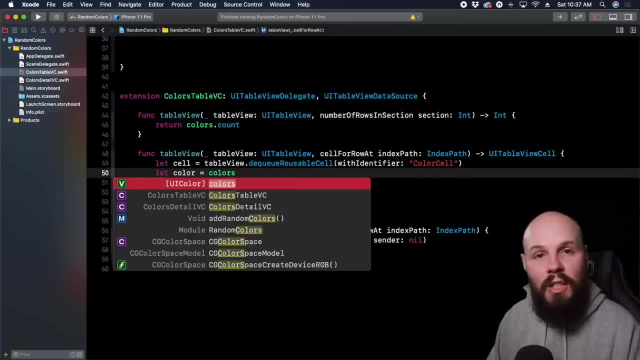 So now we need to get a color to tell this cell like what color it is. So let's say: let color equal and we're going to do colors. This is how we can access a certain location in the array. So here's where we would pass in an int. 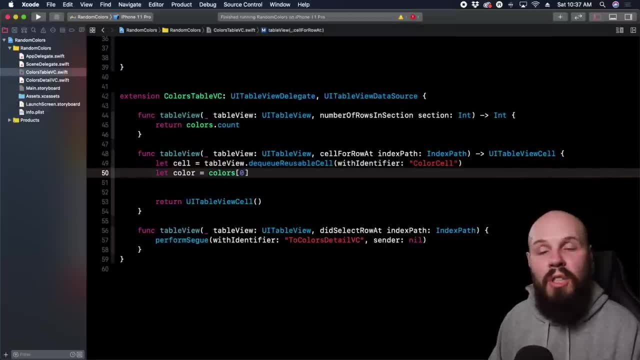 Remember I showed you this, like, if I put in zero here, this would be the first available color in our array. If I did one, this would be the second color, Two, this would be the third color, And so forth, because, remember, arrays are zero indexed. 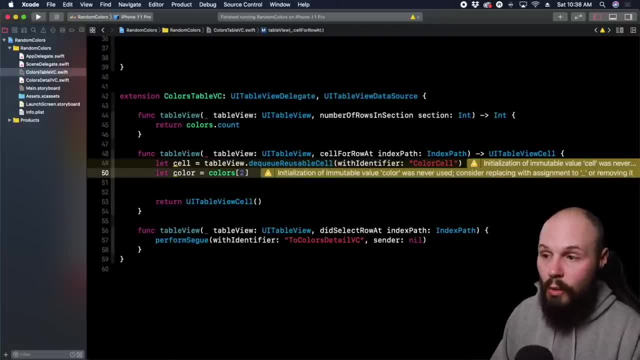 So all we're doing right here is, instead of passing in the actual int like hard coding, you know 45. No, we want to make this dynamic, And by making it dynamic we pass in index path Dot row. So the index path we're getting is right here. 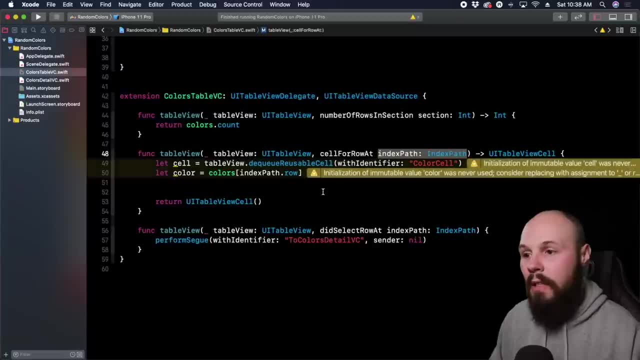 This is part of the delegate method right. Xcode knows this automatically. So, even though the iPhone is not creating, you know, a thousand cells, like we just talked about, we still do have all the index pass right, And the index pass relates to the number of cells we have. 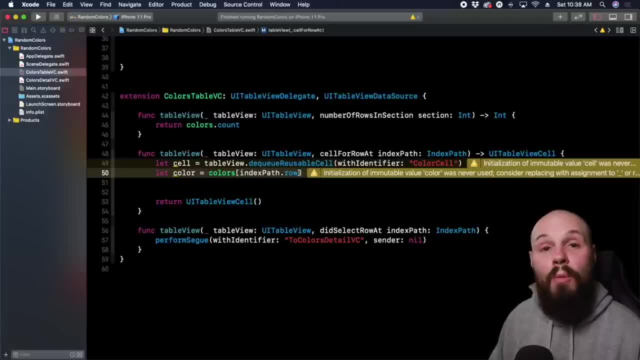 For example, index path dot row. when index path dot row is zero, that's our very first item in the colors array. So what we're doing here by passing in index path dot row is: whatever row we're on, send that number. 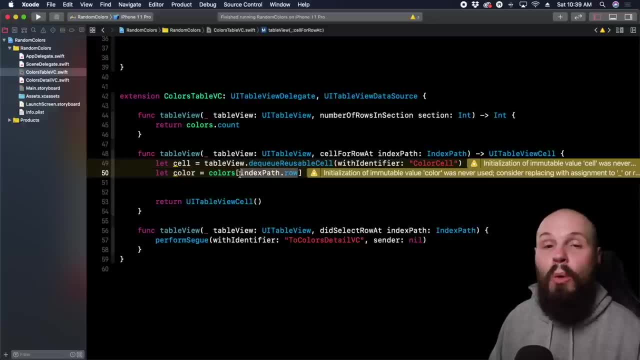 If we're on row 47, index path dot row will equal 47.. If we're on row four, index path row will equal four, And that's how we'll know what color to pull out of the array. Again, if we're on row four, index path dot row will equal 47.. 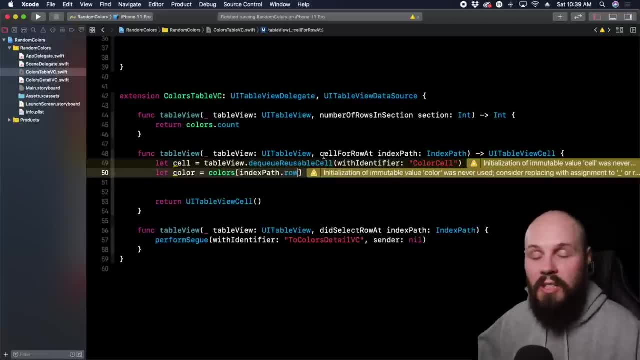 Again. if we're on row four, index path dot row will equal 47.. you know, remember this. this method is being called constantly all the time as you're scrolling, so if the one time it gets called again we're on row four, it's. 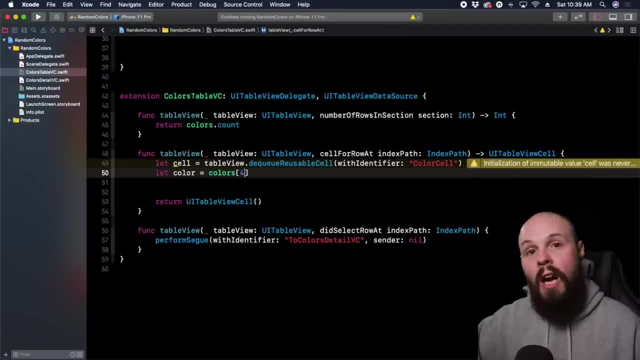 the same thing as it being like this: right, and we're gonna pull that color at that index out of the array. so hopefully that made sense. again, feel free to ask questions in the comments, not raw row in the comments or the the slack channel, because this is a confusing part. but once you understand this, you're really. 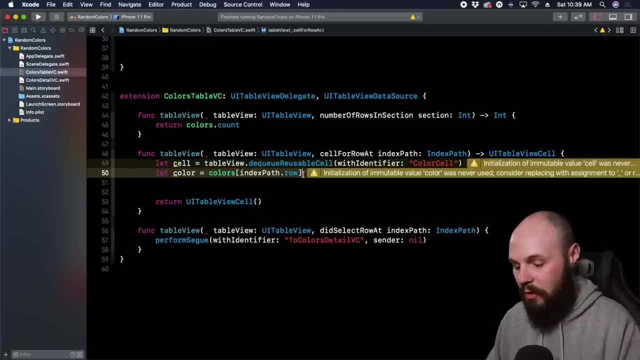 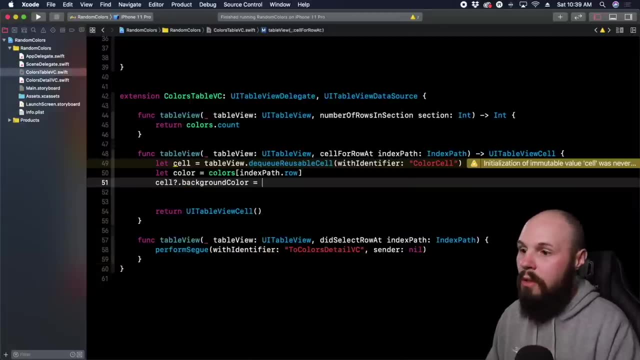 gonna understand table view. so again, feel free to ask questions, happy to explain this further. so now we have our color that we want. so now we can do cell dot. background color equals color, the color that we just pulled out right here and in fact, if you wanted to like, I broke that out so you can see what was. 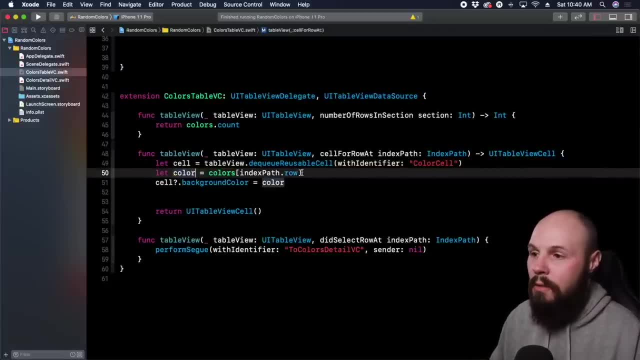 going on. if you wanted to write this code- you know smaller- you could just do: background color equals colors, that new expat, that row, and not even have this line of code, and that's probably how I would write it. you know, if I was writing the, the. 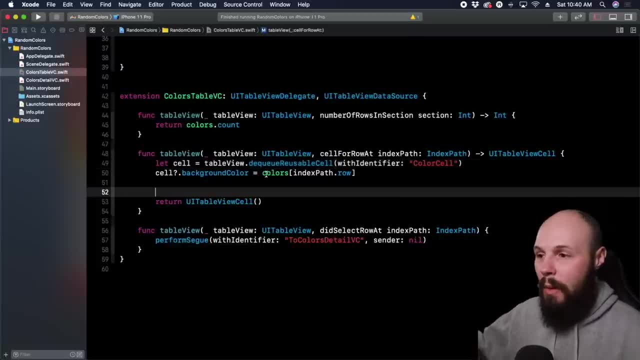 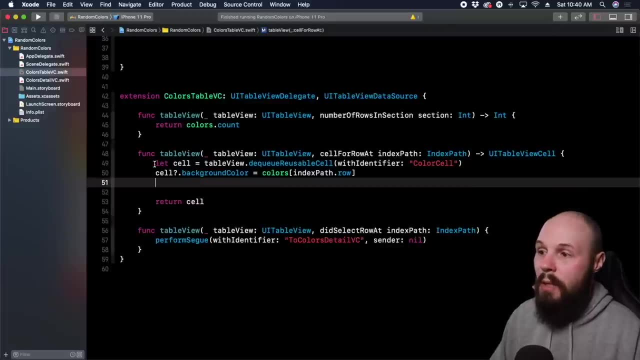 the, a real code base, but I wanted to break the steps out so you could see what was happening. so now, instead of returning just a blank normal table view cell, we want to return cell. remember this, the cell that we created up here on line 49, and then we told it what background color to be. and then now we are. 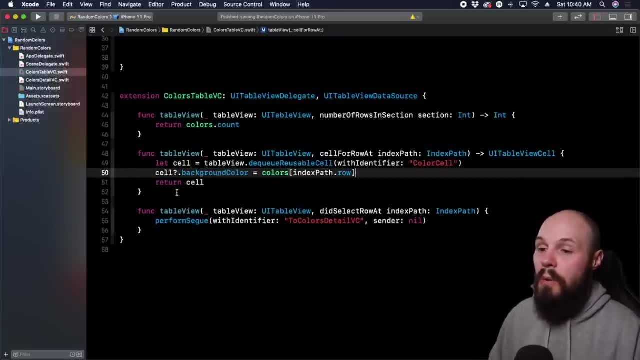 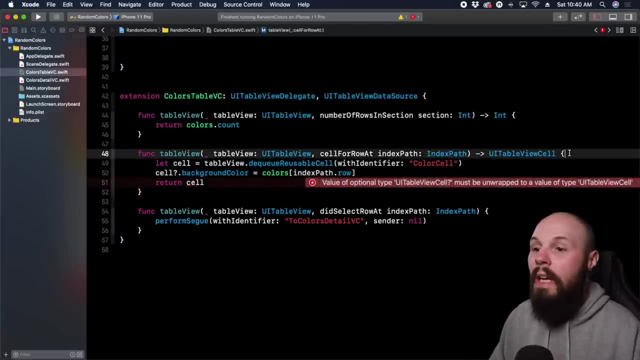 returning that cell. so I'm gonna tighten that up right here. so now when we run this, we should be getting: oh, it's an optional, so okay, good, good call there Xcode, forgot to do that. so here this returns an optional like: let me actually retype this and slowly see if I can get it back. so I'm going to go ahead and 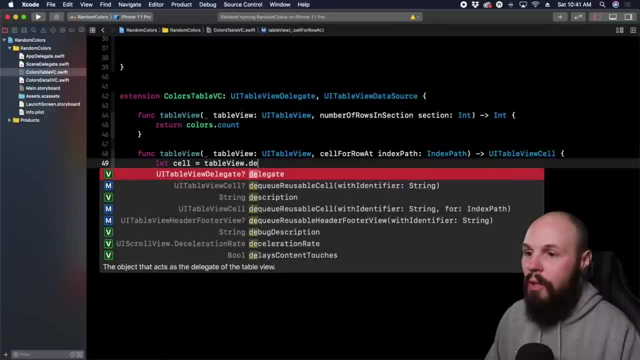 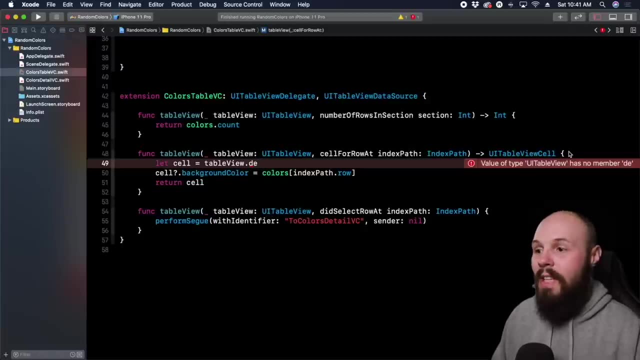 retype this, and slowly, so you can see it, so I can do table view dq. reusable cell with identifier. you can see right here that cell is an optional in case it doesn't exist. so if you want to be again, the easy thing to do is just do bang. 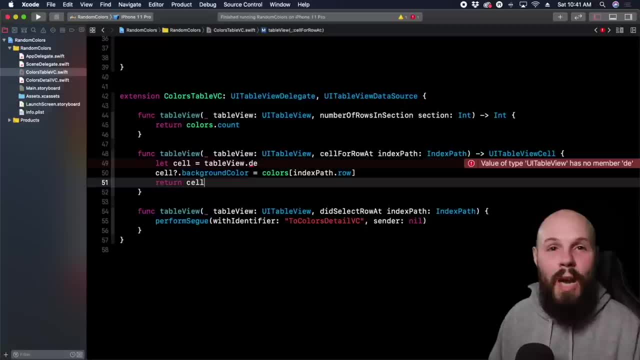 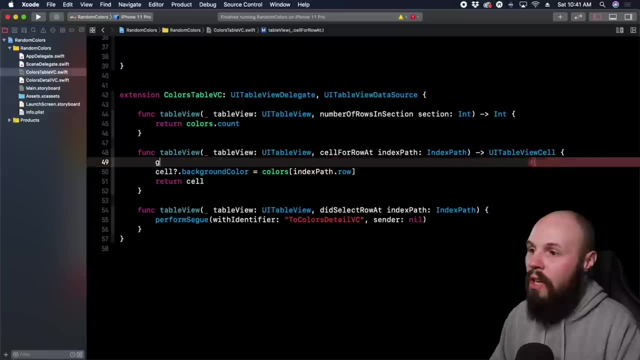 because we know it's going to exist. remember, that's the lazy way of force unwrapping the optionals, and you're gonna see developers do that, you're gonna see that in code bases, but we're gonna do it the right way real quick here. so what we should do is guard. let's this how we're gonna unwrap the optional. 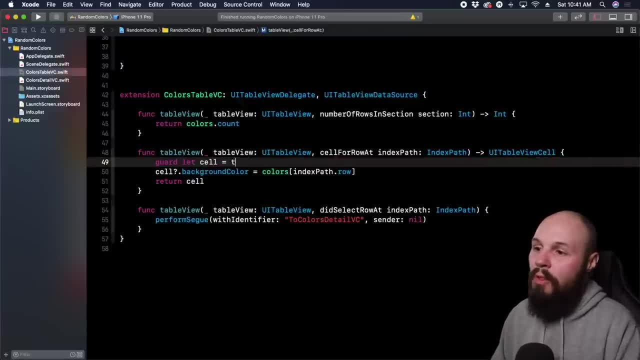 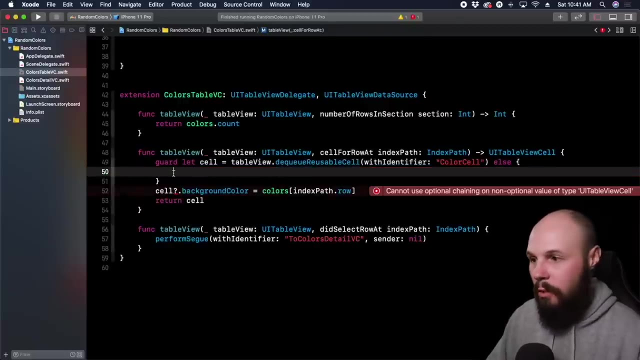 cell equals table view: DQ reusable cell with identifier string. and then that string we're going to pass in again was color cell- hoping i don't make a typo here- and then else. so this is what happens if this is nil. this is, this is the power of the guard statement. a little bit of a review here. we can return uh. 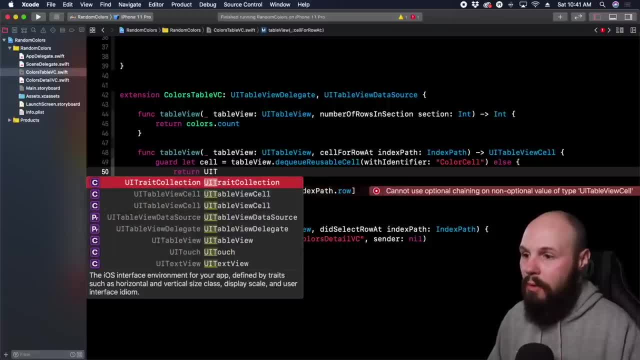 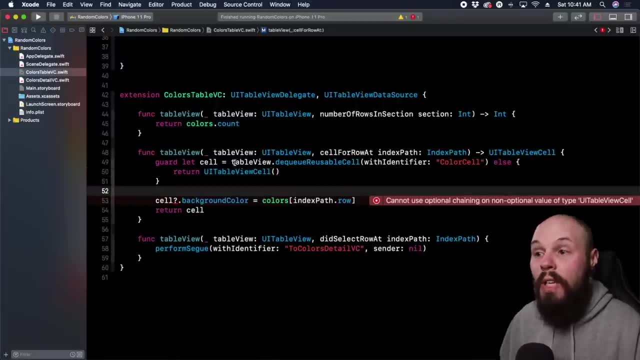 just a blank ui table uh view cell and it'll just give a blank one, but it won't crash. the guard statement allows us that early exit right, that return. so again, if for some reason our our cell with identifier color cell is nil, like say in our storyboard, we accidentally delete that cell. 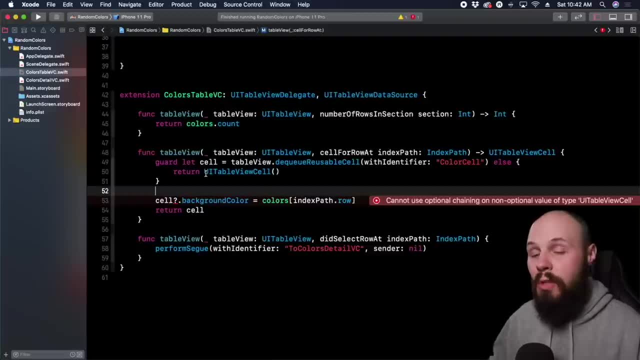 um, this will still. the app's not going to crash, which is what it would have done. um, it will just return blank table view cells. still not the uh experience you want. but your app's not just going to crash randomly and you have no idea what happens. so again the way, the guard statement. 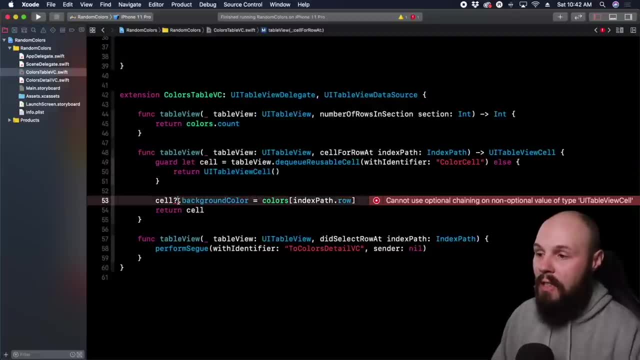 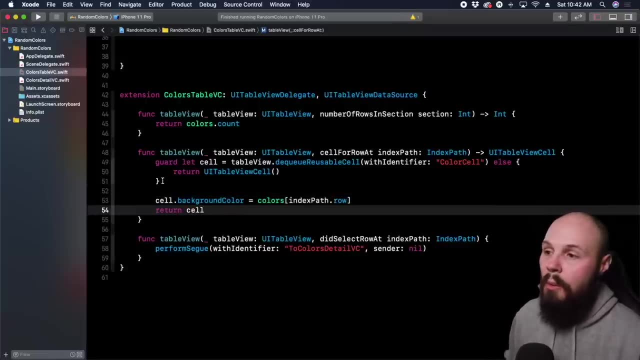 works is now that we've declared cell. uh, we have access to cell out here, like we already used, and i don't have to, you know, make it an optional. and now xcode is not going to tell me to unwrap the optional you, Because we unwrapped cell up here. so a little optional review there, um, so let's run this and 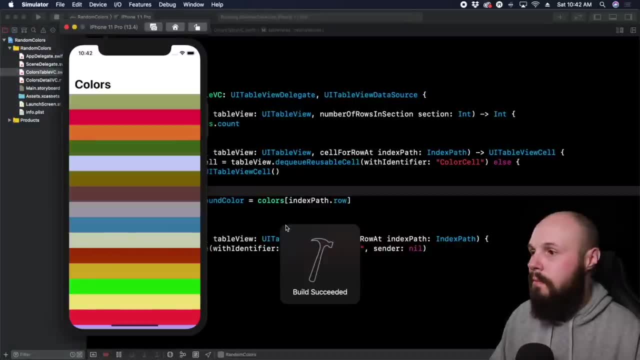 uh, we should get random colors in our array. there we go, yep, random colors, and as we scroll, 50. so what i was talking about here, like the dq reusable cell, like. so there's 1, 2, 3, 4, 5, 6, 7, 8, 9. 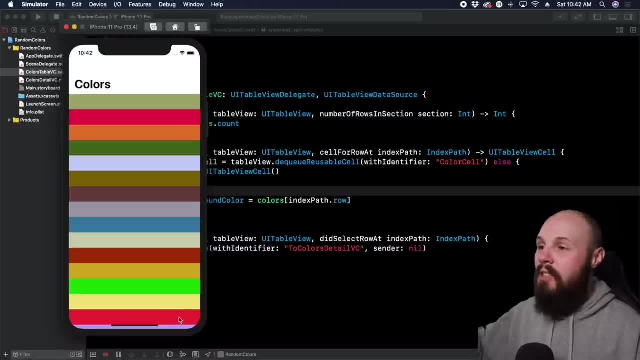 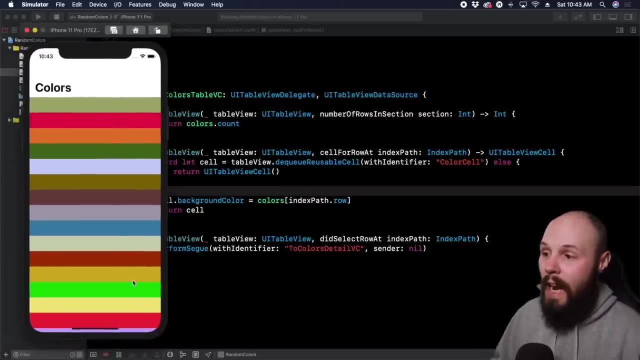 10, 11, 12, 13, 14, 15, 16- hopefully i didn't miscount that- 16 cells, right? so this, this uh self-road index path function, right- was called 16 times in the beginning and then, as i'm scrolling, it's constantly getting called. it's getting called, it's getting. 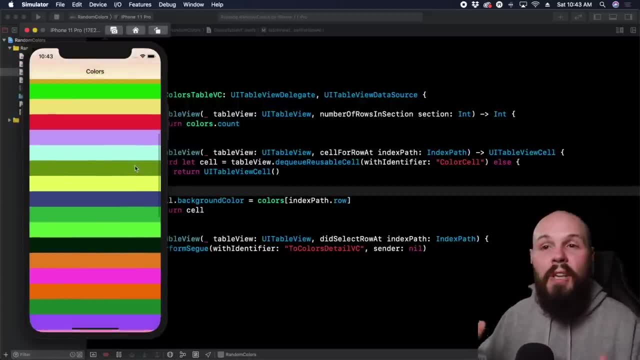 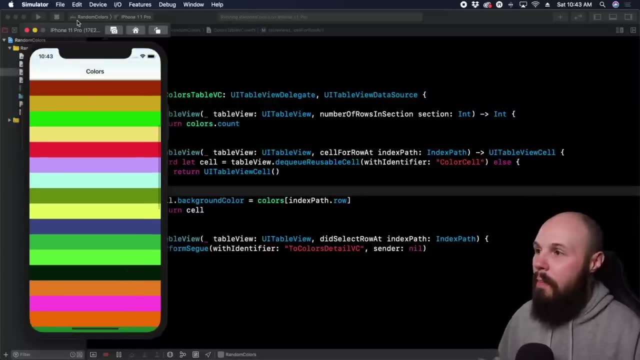 called and we're setting the background color to that cell, but again, we don't. we're not creating a thousand cells, we're only creating the cells we need, and that's for performance reasons. um, and again back to the um, remember our constraint. we wanted to constrain the bottom, not to the safe. 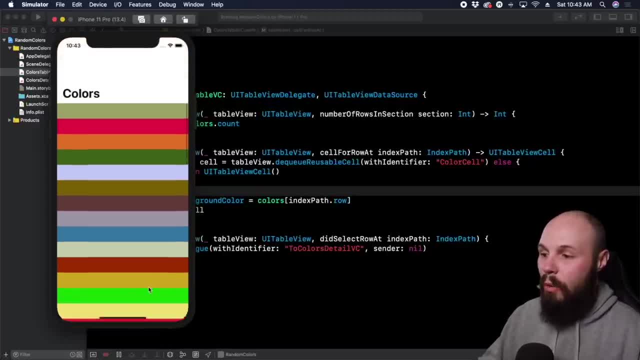 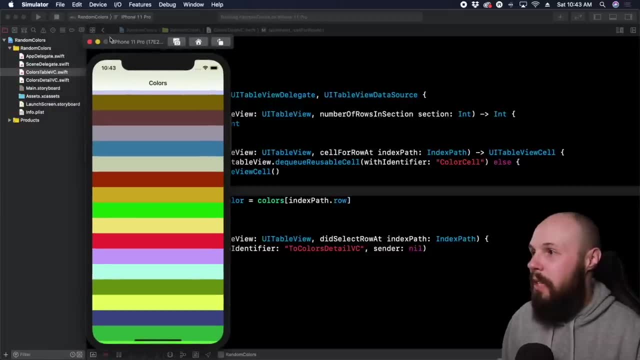 area. we wanted it to fill up the whole bottom view. i just think that looks nicer how we're filling up the whole view, whereas if we put it to the safe area right above this uh home screen, let me actually show you that. um well, you'll see what i mean by. it's not going to be the same as 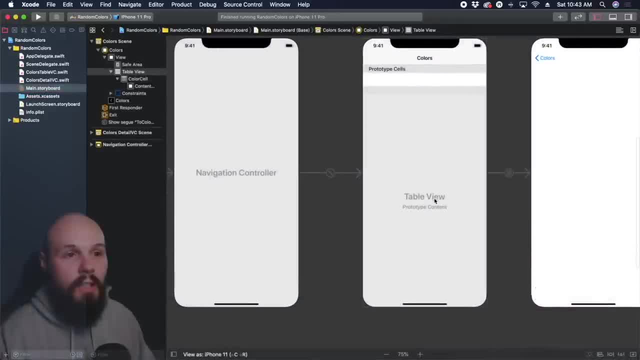 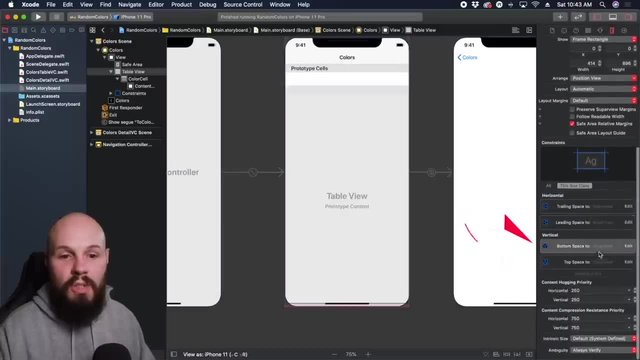 by. it doesn't look that great, and i'll show you how to edit constraints here too. so, clicking on our table view, opening up the right pane, click on the ruler to the right of that. you can see our constraints down here. so you see bottom space to super view. let's actually delete that. and now. 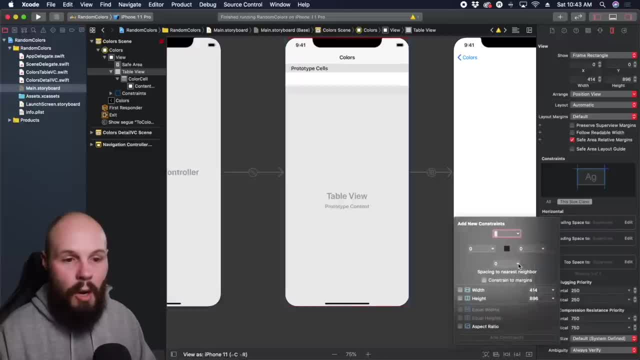 we're gonna have to create that again. uh, so let's do bottom space. whoops it's. it's got to be. it's kind of content aware, like it knows it's below the safe area. so we move it, drag it up a little bit. now, when we pin it to the bottom here we have the safe area as an option and we 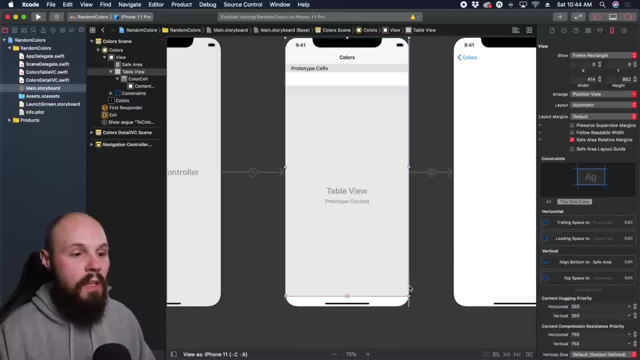 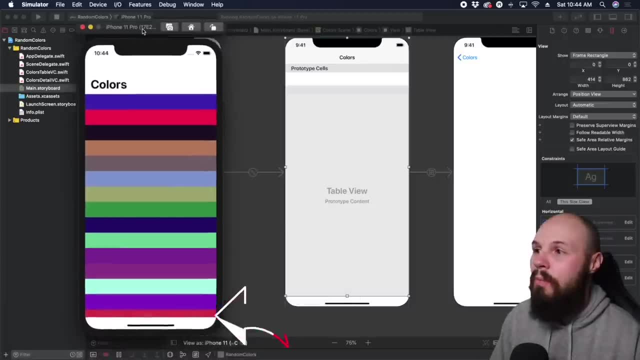 want it to be the safe area and zero. so add one constraint. you see how it stopped right above our home button. now watch when i run this and you're going to see this with all your table views and i always recommend pinning them to the view most likely. but now you see, when we scroll, we always 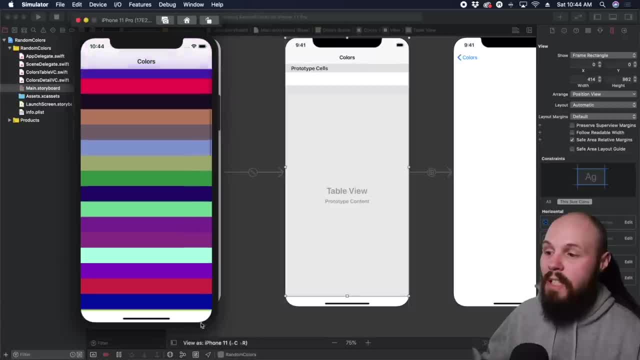 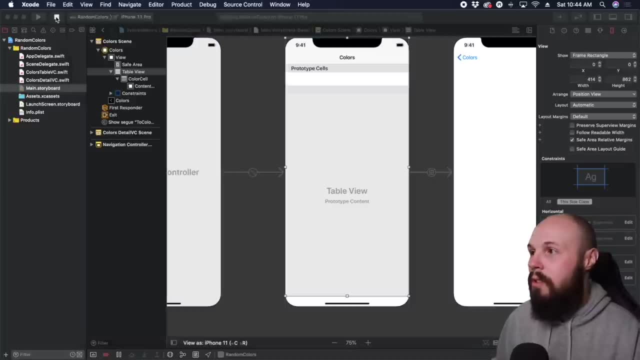 have that like white bar at the bottom because we pin it to the safe area. so that's an example of the safe area on the bottom. again, i think it looks cleaner and nicer when all of our colors, like, fill up the whole screen. so let's, let's do that again here, so again we can delete the align bottom the. 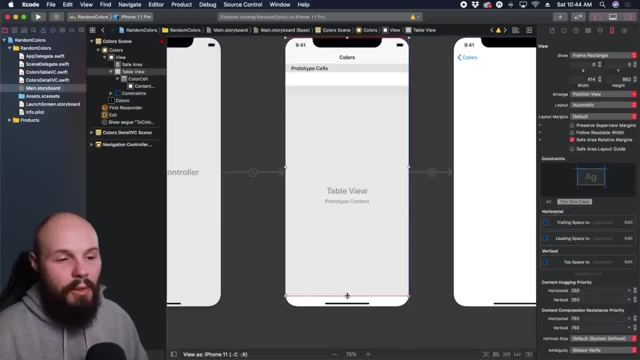 safe area. delete that and i mean you can probably see that it's not going to be the same as the edit it. i always find it just safer to just delete it and redo it. um, so again the bottom we want to pin to the view, not the safe area in zero hit. add one constraint now when we run it. 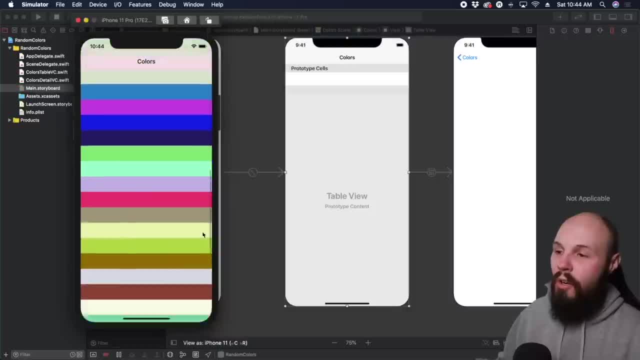 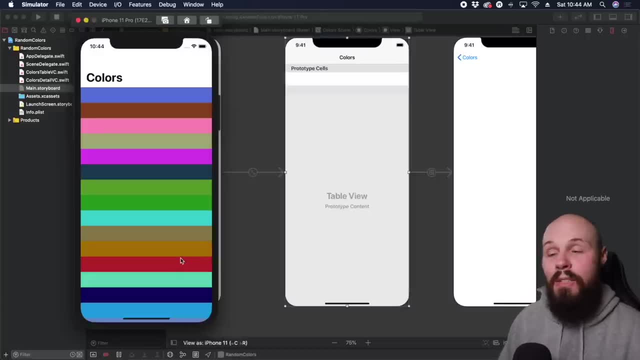 again. um, you're going to see how it just looks better, right, it fills up the whole phone. um, just looks a lot better than that. so now, what we haven't set up is, uh, passing the data to the next view controller. so watch, when i click a color, we're just white because we're not actually. 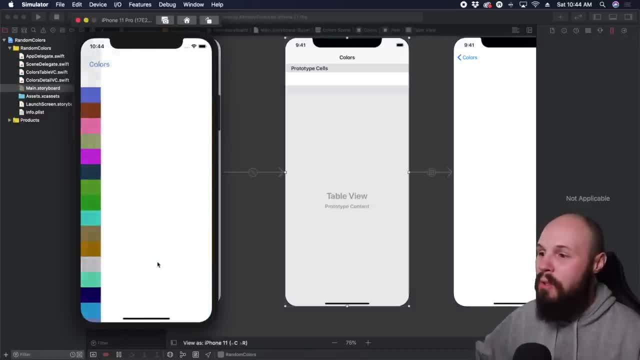 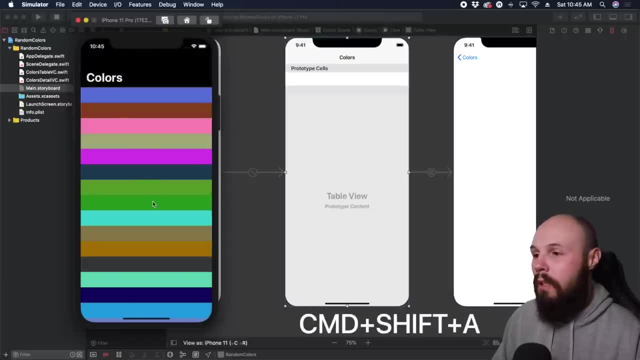 passing that data. um, so that is the final piece of the puzzle, if you will. oh, and also a new, uh fun shortcut command: shift a on your simulator. we'll change the dark mode real quick. thanks to jason for pointing that out. uh, so you can test it. what it looks like in dark mode. 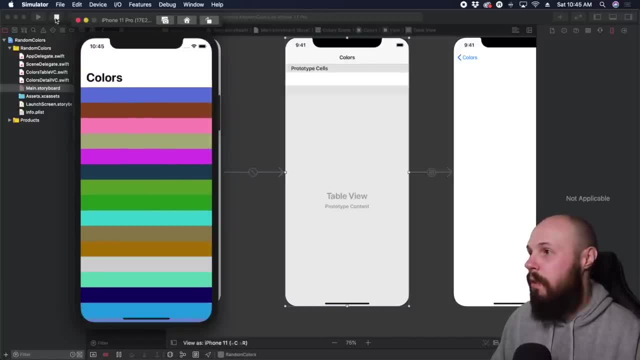 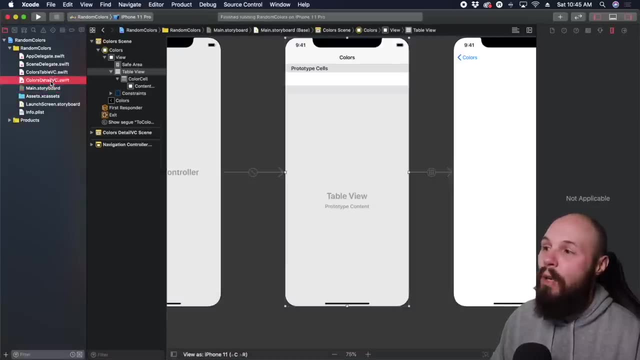 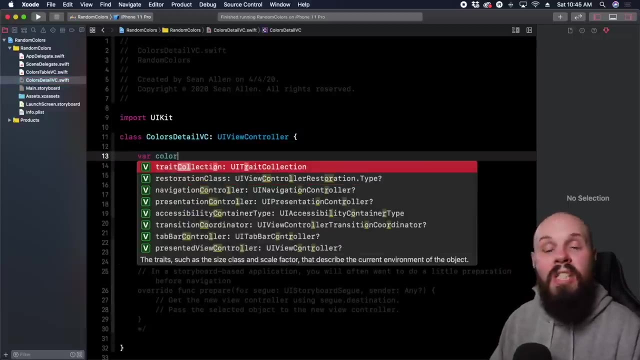 and then command shift a to go back to light mode. a little fun fact there, okay, so now let's work on passing the data so back into our uh. well, actually let's go to the color detail vc first. so what we need here is a variable called color, um. so let's do var color now. we're not initializing it with. 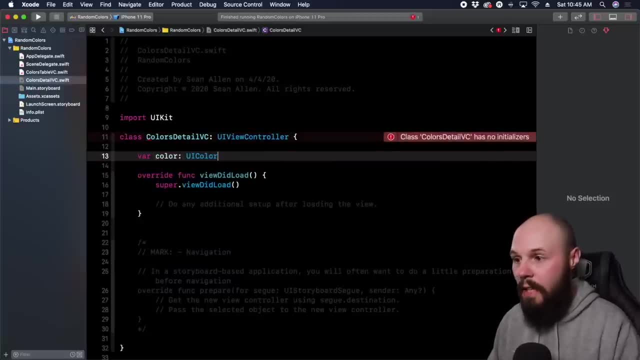 anything, a specific color yet, and say this is of type ui color and it's an optional um, because we're waiting to pass the data right. this detail vc is waiting to receive, receive what color it needs to show. so that's why this is an optional. if, for some reason, you use this view controller and it's not receiving a 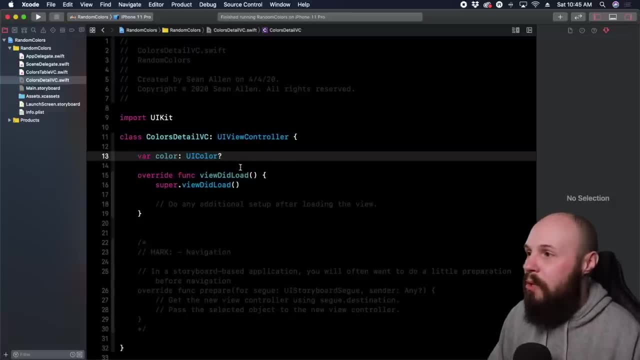 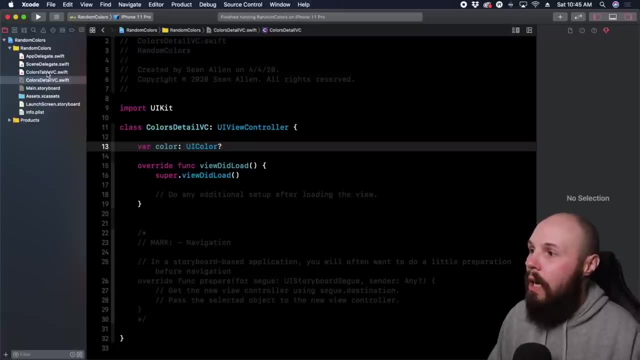 color. you don't want to force unwrap it just in case, um, so make it an optional, and then? so now our colors detail vc has this variable called color. so in our uh colors table view here in did select row at remember. this is what happens when we tap on it again, we can create our color. 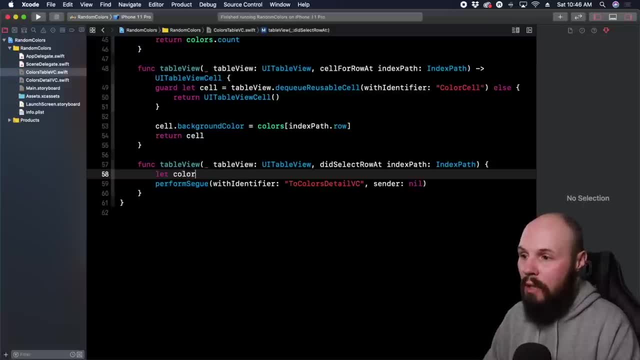 just like we did uh above here we can do: let color equals colors, uh, and then again, uh, what we're going to access? right, we don't want to access four or five, we don't want to like hard code that we want to do the same thing. index path, dot row. so again, this is whatever row we tap, that's. 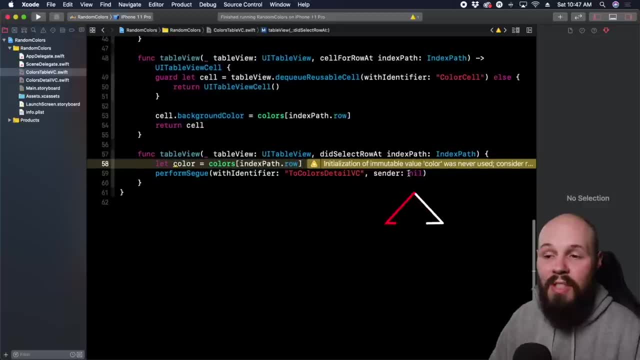 the number we're going to pass into our color. and now, remember, before i said we don't have a sender yet. so now the sender in our segue is going to be color. so now, whenever you're doing some custom stuff in your segue you have to write a little bit of color and then you're going to have to. 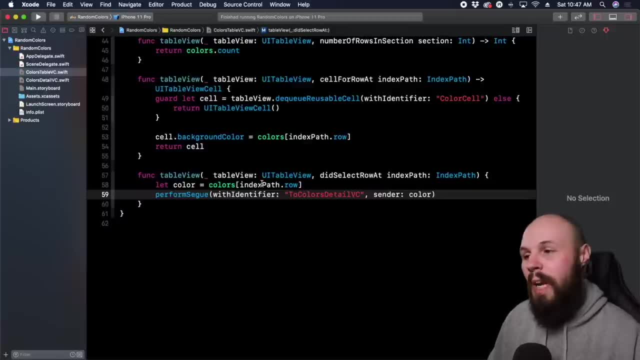 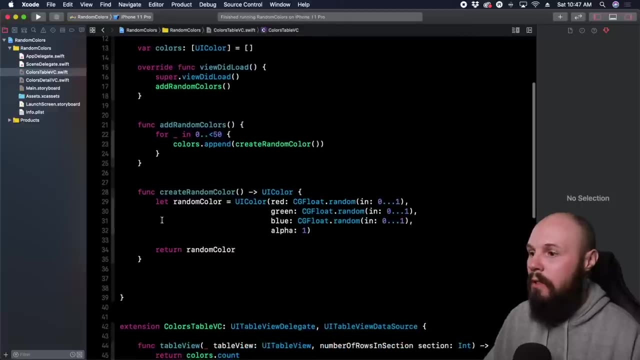 code to handle that. before we didn't, because we were just showing the screen, we weren't passing any data. so the code that handles your segue is a function and we're gonna do this up here back up in our view controller. uh, let's actually clean up some space here. 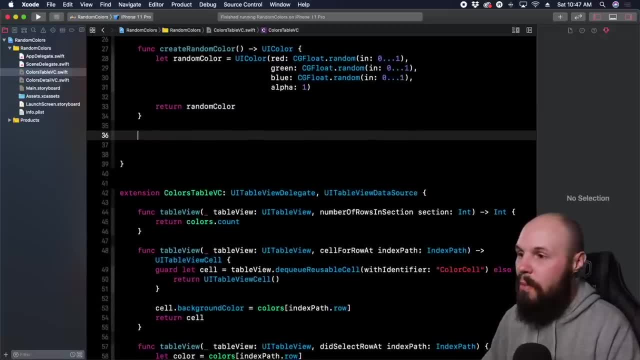 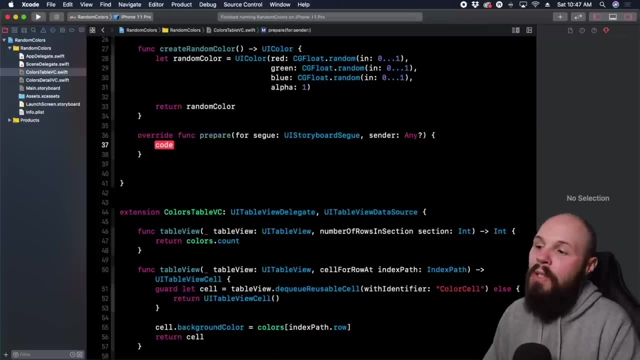 is a function called uh, prepare for segue. so if you start typing prepare, this is already built in and you can see we get it down here: prepare for segue, and here we need to like designate our designation. so i always call this dest vc for destination vc. so let dest vc again. 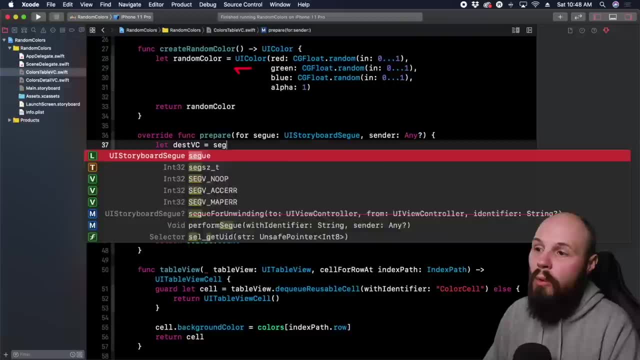 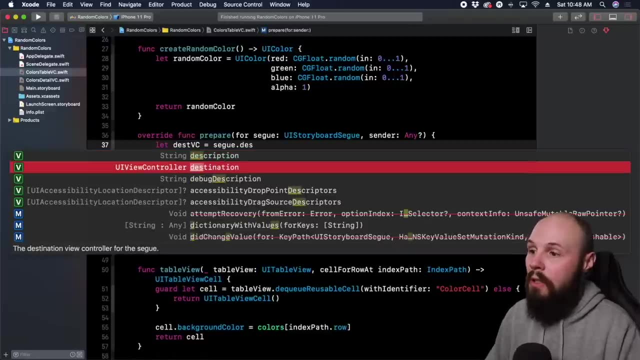 short for destination vc. uh equals you can do segue because we have this being passed in as a parameter. so our segue has a destination: uh view controller. here that is a property, so segue dot destination. now, so this is saying wherever our segue is pointed to. that's what. 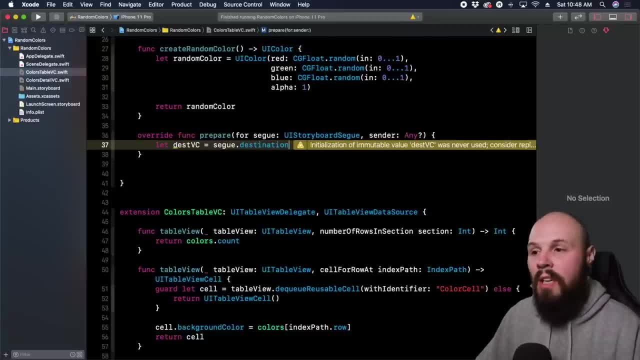 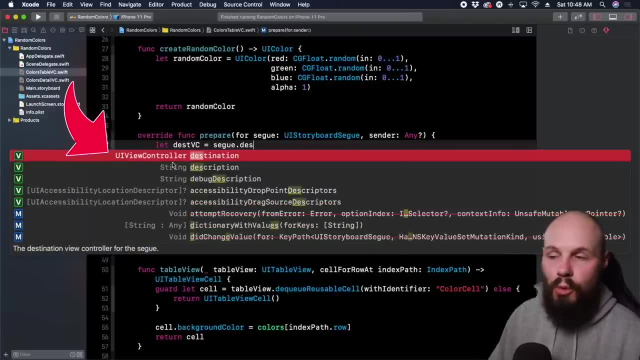 i want this desk vc to be and we want access to this so we can set the color. and the thing is like: let me delete destination and you'll see what i'm talking about here. you get that destination, you can see it is up. type ui view controller. so that's just a generic ui view controller. 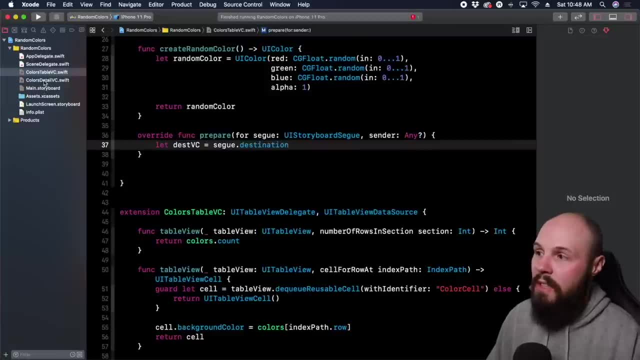 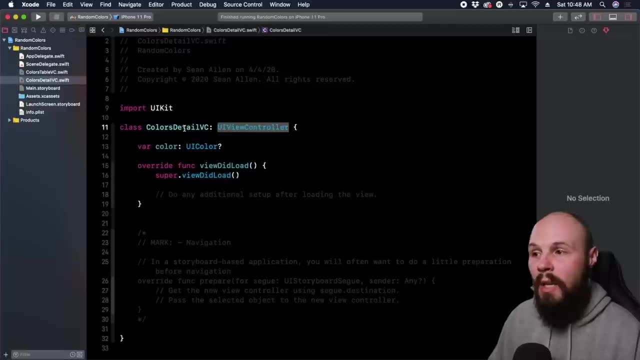 not our custom one. now, if you remember, back in the colors detail vc we have our specific colors detail vc. that's a subclass of ui view controller, and this colors detail vc- that's a subclass- has a special variable called color that not a normal view controller doesn't have this color variable. 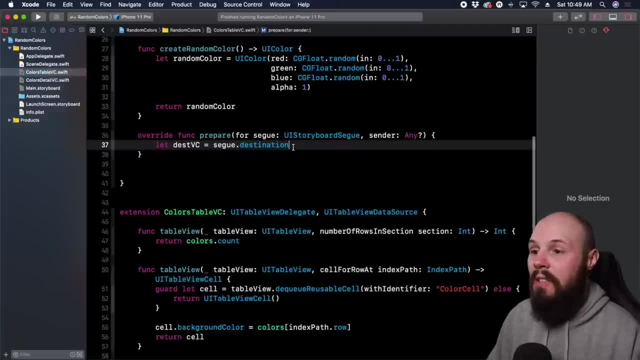 that we put in. so back in the table vc, i have to- uh, this is called casting. i have to cast this regular view controller as a colors detail vc and by doing this this is letting uh this view variable know: hey, you are of type colors detail vc. and once i know that, i know that i have access. 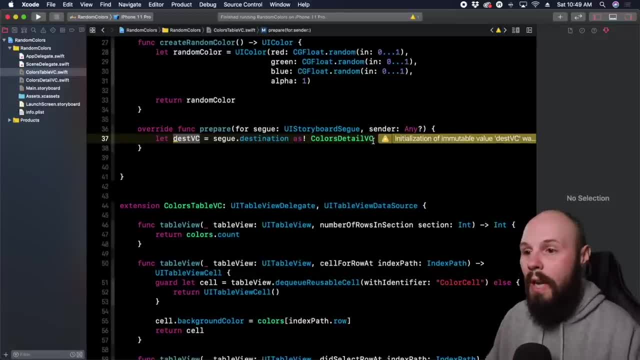 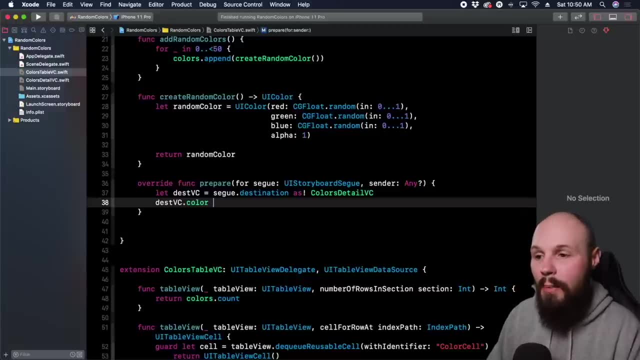 to that colors variable that most normal view controllers don't have. so now i can do des, vccolor, and you see it's an optional um. and now i have access to that color variable again because we've casted it as a colors detail. vc equals sender, uh, and you see sender when i type that. let's do that. 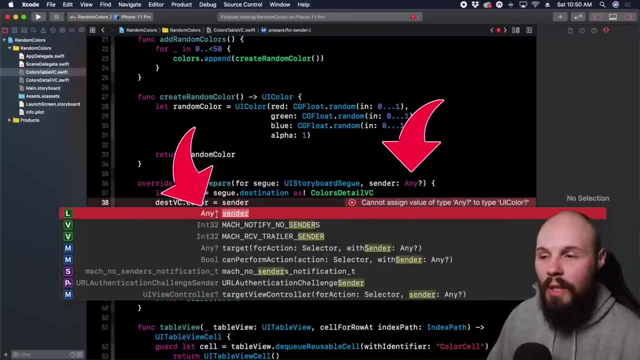 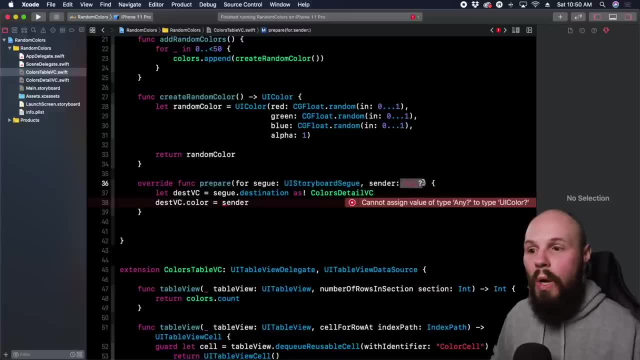 sender is of type any. um, we won't get into this quite yet, but i'll give you a high level overview. when i pass in a sender, that means it can be any type. but when you pass in any type, what? what this function is basically saying is like: hey, just give me an object, i don't care what type it is, but when? 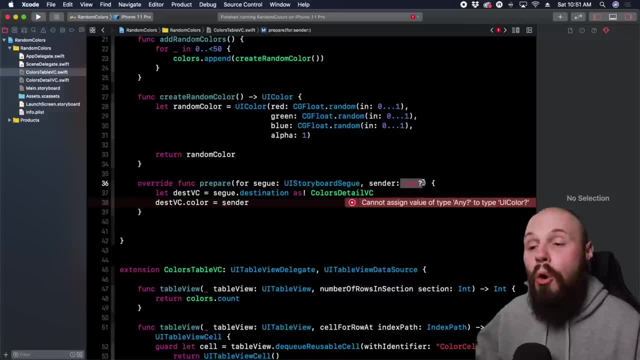 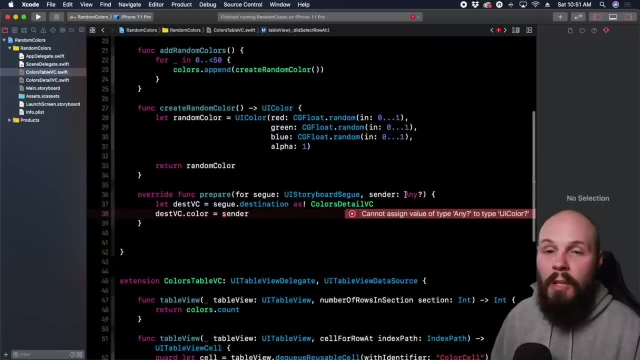 i give you this object back, i'm not going to tell you what type it is. you have to know what type it is. so again, by passing color down here, as the sender, we pass it in, but when we use it up here we have to say, okay, this is a ui color as a ui color, so let's run through that real quick. what? 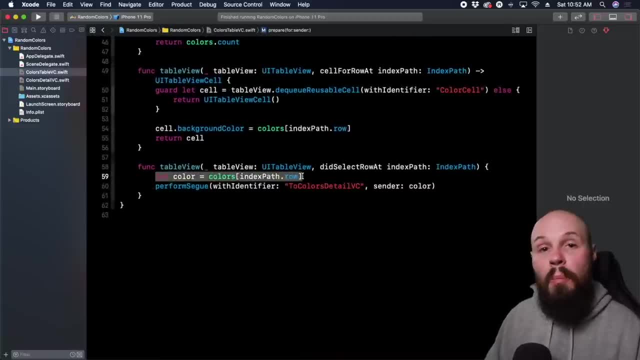 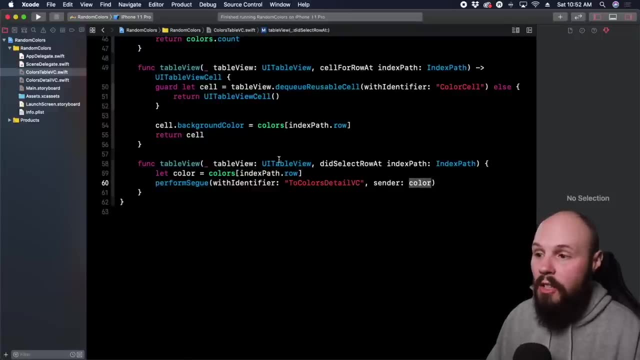 happens when i tap the row. we're going to get the specific color based on the row that i tapped. that's what's happening here- and then we're going to perform the segue with identifier and then we're going to have a sender of the color that i just created right here on line 59, so that also. 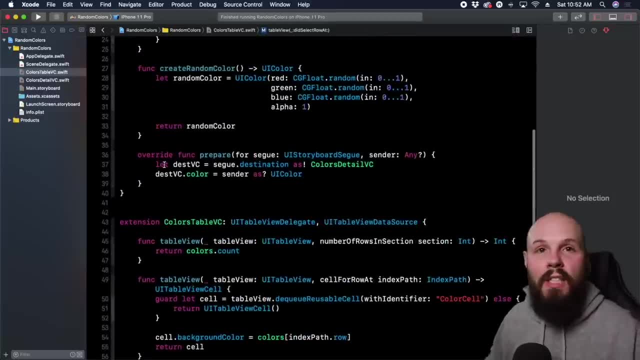 kind of triggers. this prepare for segue. so we're creating a destination view controller. we have to cast that regular view controller as a colors detail vc so we can get access to the special properties of the colors detail vc, which in this case is just color. and then we are setting the. 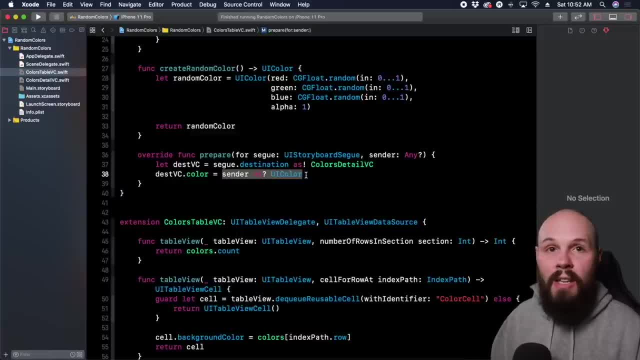 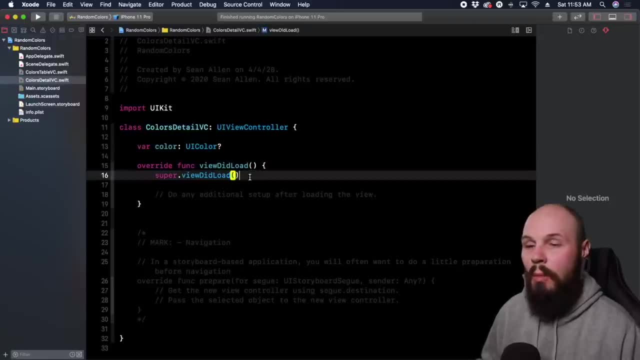 color here on this destination vc as the sender that we passed in the random color that we tapped. now if we go to our color detail vc, we're going to have this color passed, but we have to use that color right. this is passing the data. we pass the color from the. 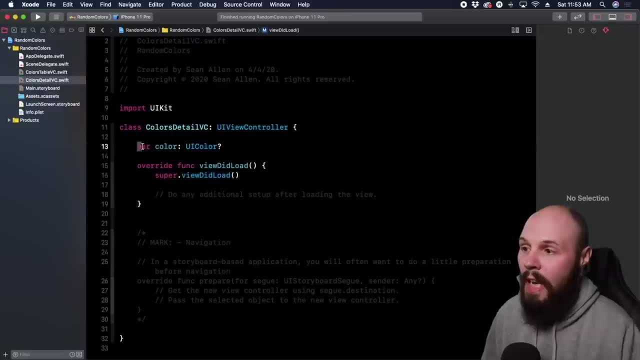 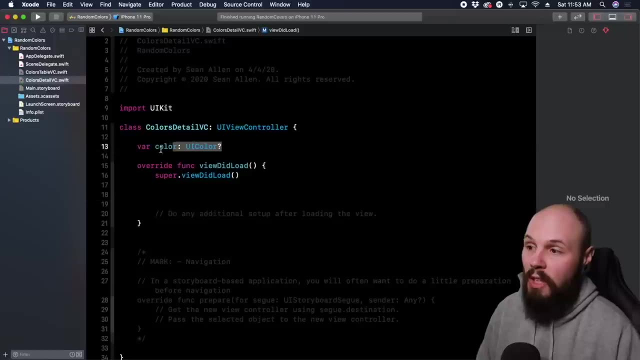 table view screen to our detail screen and that is going to be captured in this variable called color. so now what we need to do is use that color. so we need to unwrap because this isn't optional. so we can do. we'll do nil coalescing right now, just to show you the various ways that. 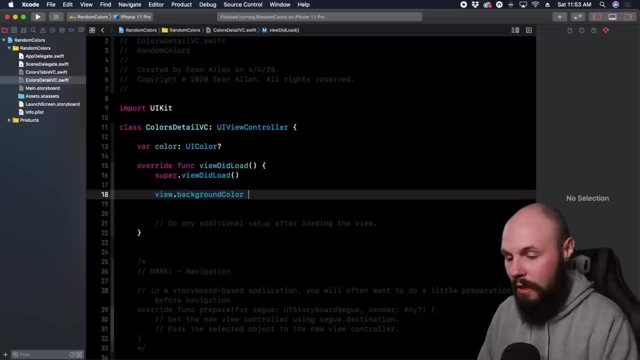 you can do that to unwrap an optional. so we can do view dot background color equals color. that we the variable right here. but you're going to see it's an optional so we need to give it a default value. remember this is nil coalescing. so this is saying: 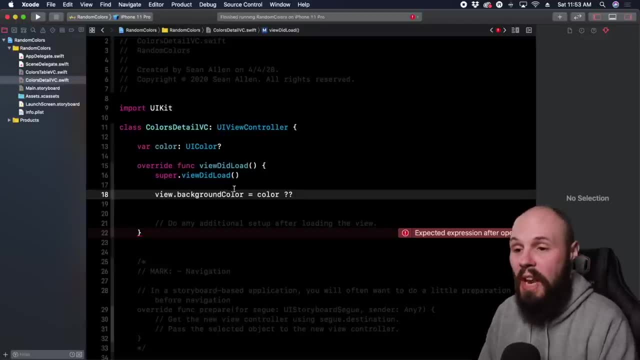 if color has a value, use the color we pass in. however, if it's nil, we're going to use a default value and we're just going to say ui, color dot, let's call it blue. um, and actually i believe we color, we can just do dot blue, because background color knows it's a ui color here, so let's get rid. 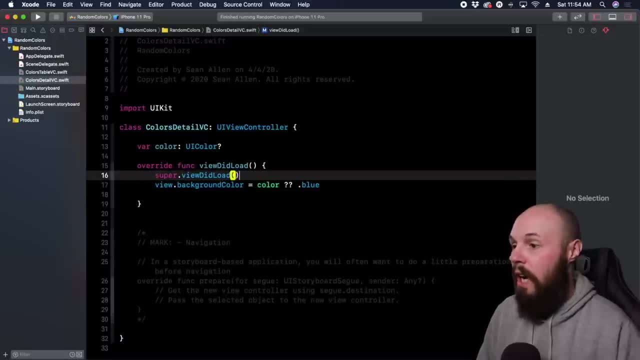 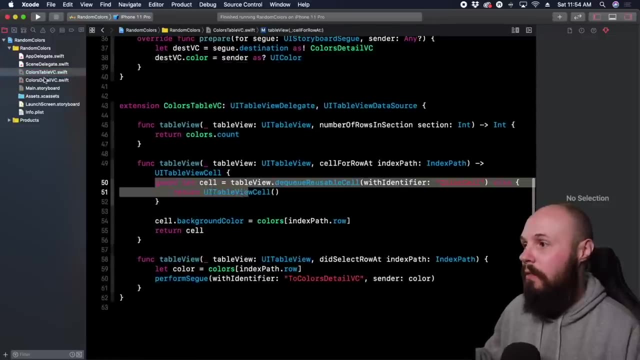 of this, these comments, this boilerplate code here, uh. so again to review: uh, you know, we've used guard let uh here to unwrap, uh, this optional and i've used, uh, no, coalescing here, uh, to unwrap the optional. you could have done it, you know, with if let. you could have done it with guard let. 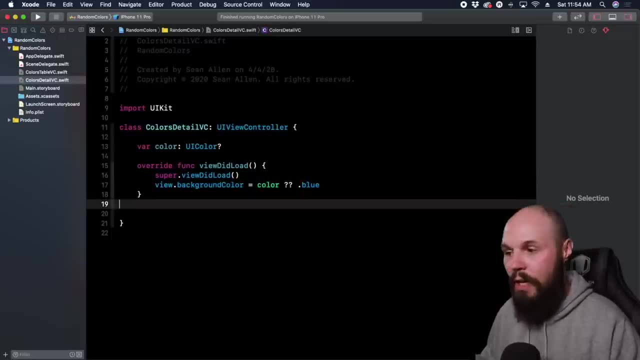 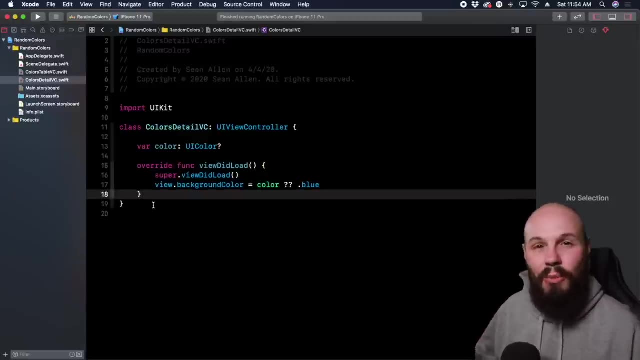 um, i know you're probably thinking right now: well, when do i use which type of of unwrapping? there's really no like hard and fast rules. um, it's kind of like: use the right tool for the right job and unfortunately, you're not really going to know that until you, you know, get more. 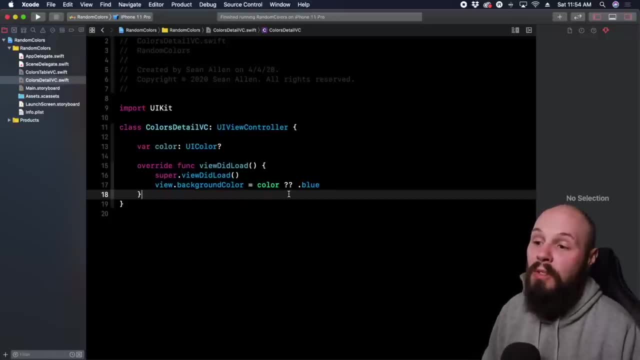 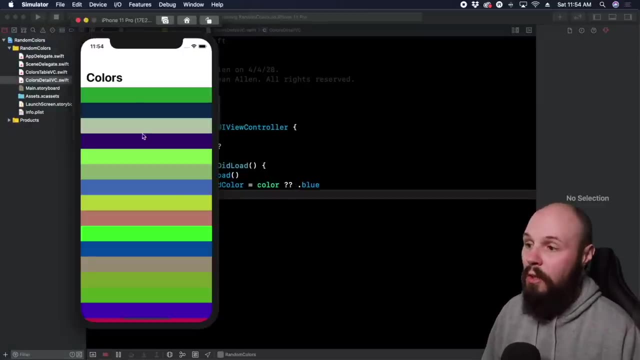 experience. but, um, you know, this is a quick and easy way to unwrap this optional here where we we want to give it a default value, right, um, okay, so let's run this and see what we get. so again, here's our random colors: very bluey, greeny here at the top. okay, cool, so let's pick. um, i don't know. 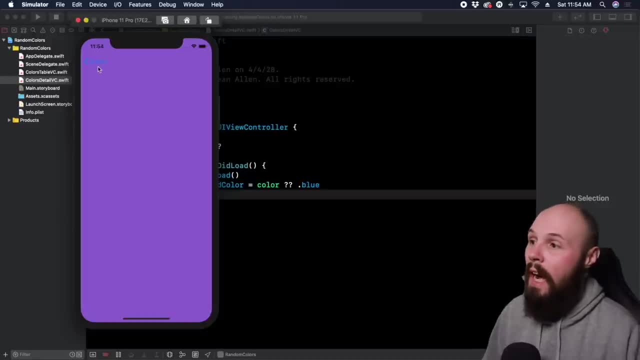 let's pick this purple right here. bam, we passed the purple here and now we have this back button with colors. uh, so back here we are, back here, back to the top. tap on this green, the very first one, and now we pass that color green and set it to the background color. now, one thing i'm not sure: 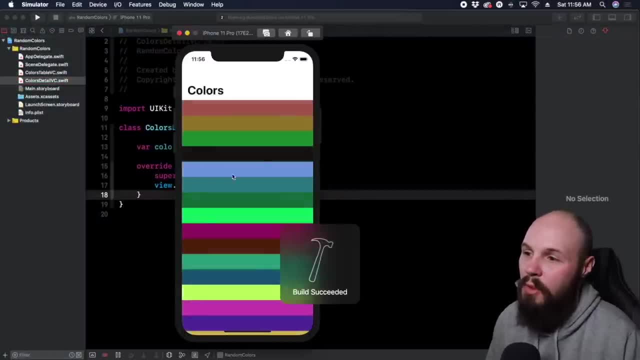 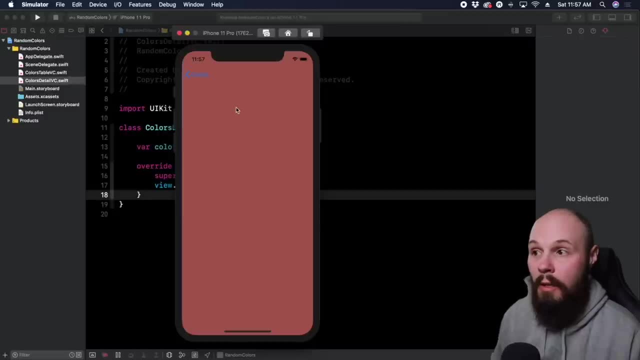 if you notice, but this may throw you off right, let's run it again. um, so you see, we have this color at the top. it's like a maroon brown, i don't know. it looks weird. if you click on it, it turns gray right and we go back. oh, now it's gray. why is that? now let's click on this green one. let's. 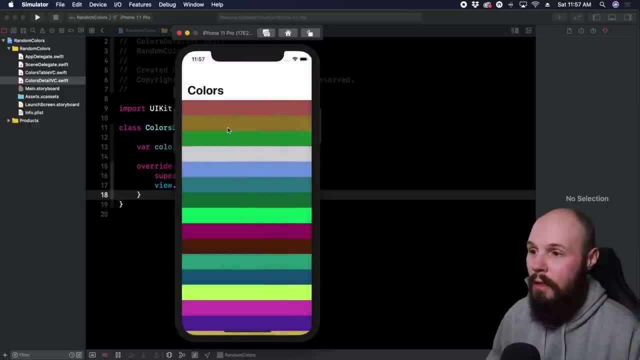 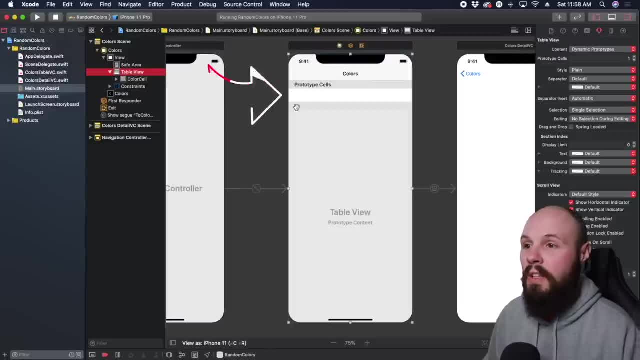 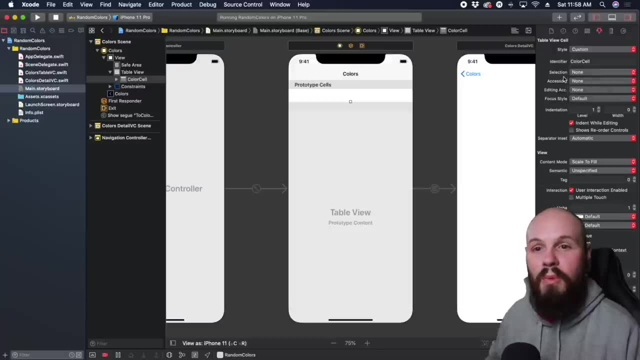 that cell. so what we can do here is in the main storyboard and if you click on the cell, uh, you can do selection where it's blue. i don't know why it's clicked on blue and it's showing up gray, but you can do none um. so that means when you tap on the cell, it's not going to turn a specific color. 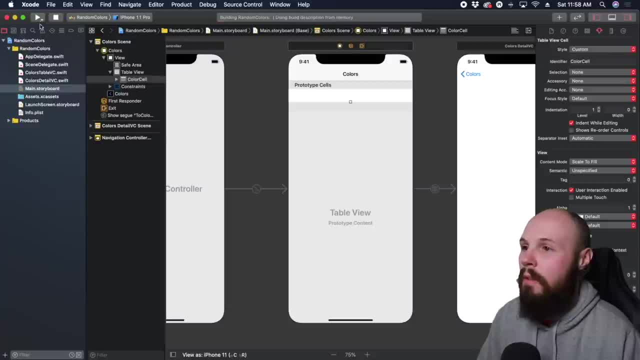 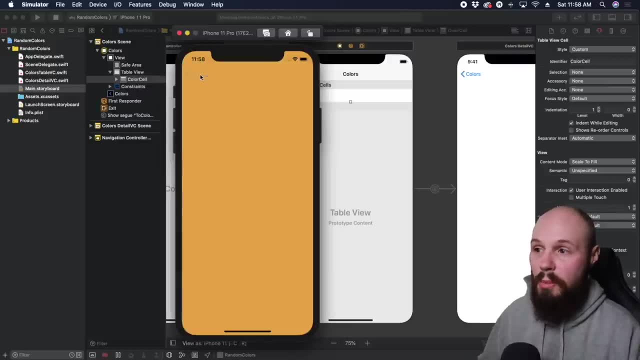 so now let's stop this and run it. now, when we tap on a cell, it's not going to change color. so let's tap on this orange one at the top. you tap on it, you notice it didn't change color, whereas before it was changing to gray. uh, let's test it again here on this purple one. 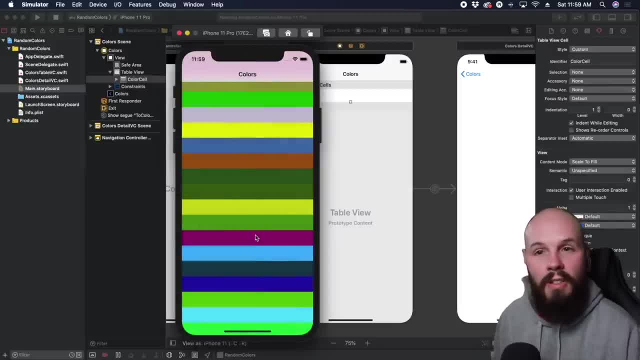 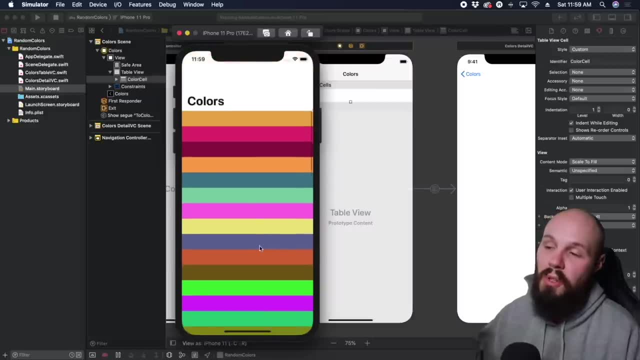 purple, back to purple. it didn't go gray and again that's. you've probably seen this in other apps, where you tap on a cell and it like turns gray to show you that it's selected. um, so that is one potential confusing thing with our colors app, because our entire cell is a color. we're kind. 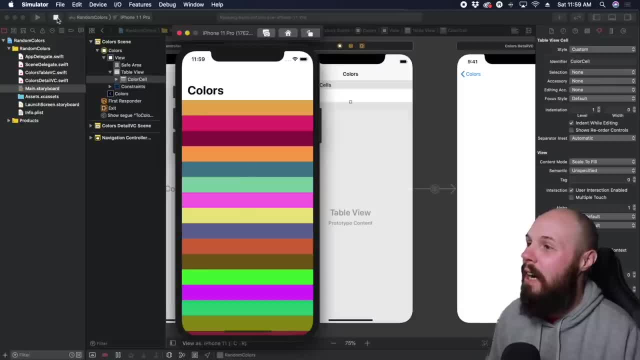 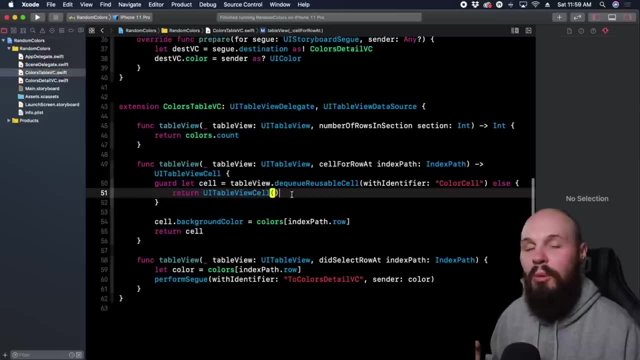 of changing the color of the cell. so one quick little fix, uh. another thing i want to talk about before we finish this video, and this is the last thing, is a little bit of refactoring, and i want to talk about this: uh, throughout the apps, to give you a little taste. 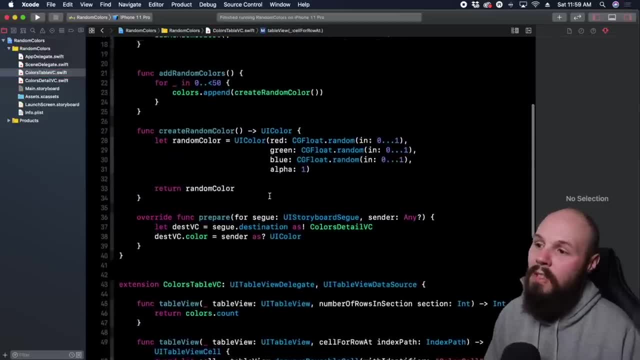 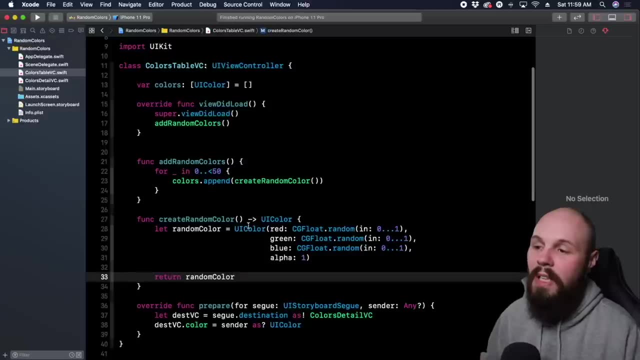 of it. uh, so what we can refactor here is this: create random color. right, this is a function um that the view controller doesn't need to know about this. we can make an extension on ui color, so we can do ui color, dot random, right, you know, like, how we do ui color, dot blue, dot, red, we can. 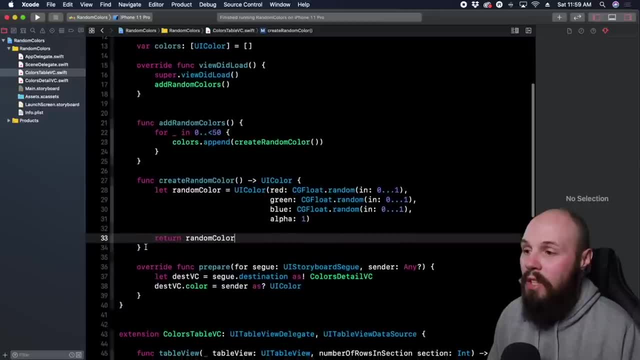 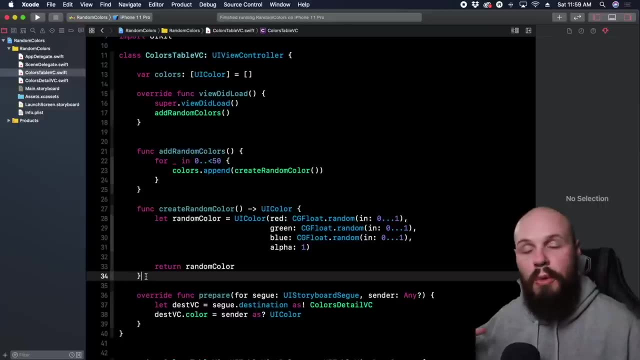 dot random. that way it spits out a random color and we can get this function out of our view controller. and it also makes that code reusable no matter what view controller or screen we're on, whereas by putting this code in the colors table, vc, this code is only accessible in that vc. well, getting a random color. 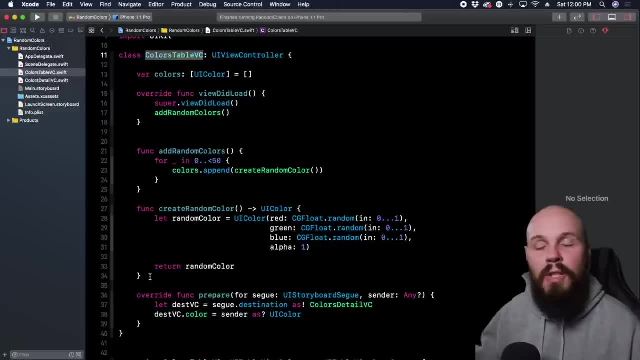 i don't know, maybe we're doing a big time colors app. maybe we want to use that throughout our app. so let's create a colors extension to add this functionality to ui color and not have it be contained to our- our colors table, vc. so here in your folder, do command n for new file, this time. 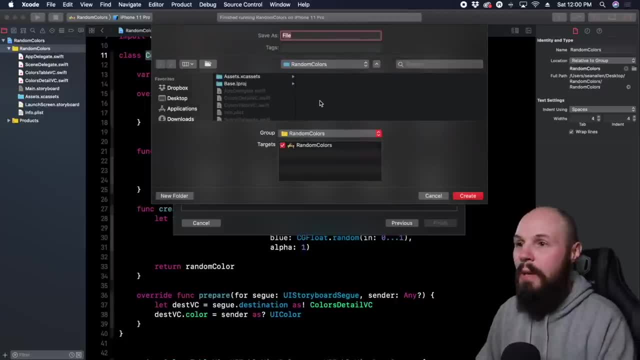 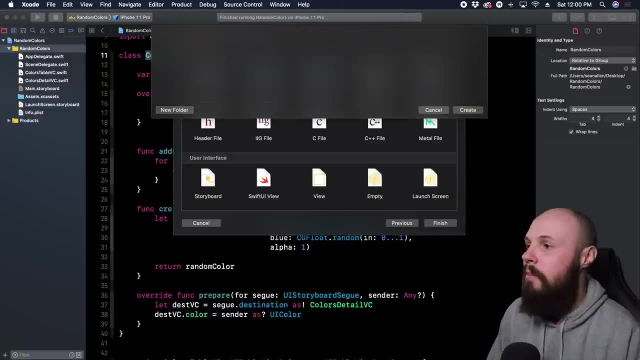 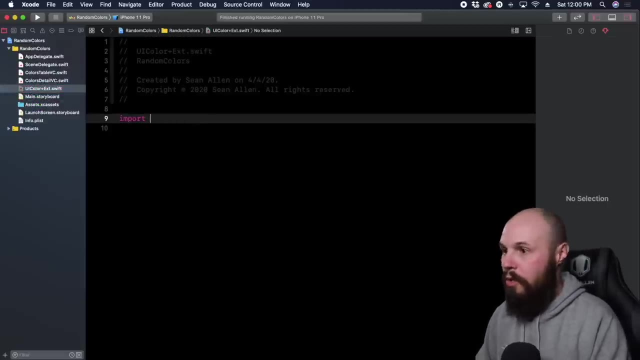 we are going to do a swift file, hit next, and i always name my extensions, the, the type. so ui plus ext. for the extension. hit create. now you see, we have colors plus ext and here we need to import ui kit because it's ui color, remember. so import ui kit and just so you. 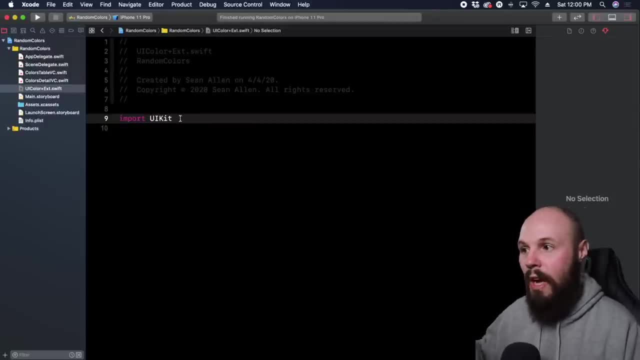 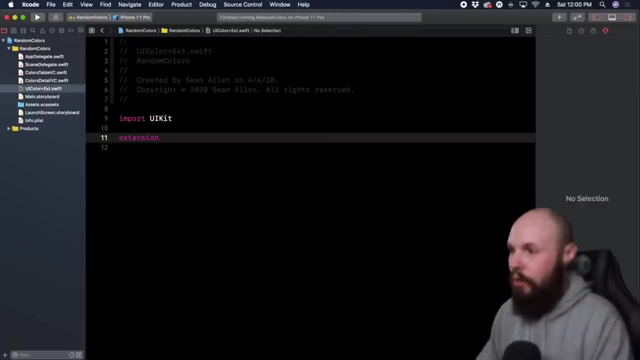 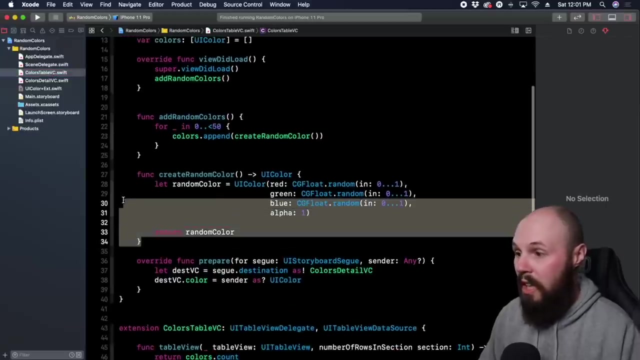 know ui kit also imports foundation. so if you have import foundation and import ui kit, that's redundant. so here we can do extension, ui color and here's where we can add some functionality. so let's go back to our table vvc and we're just going to literally cut and paste. we got to make a. 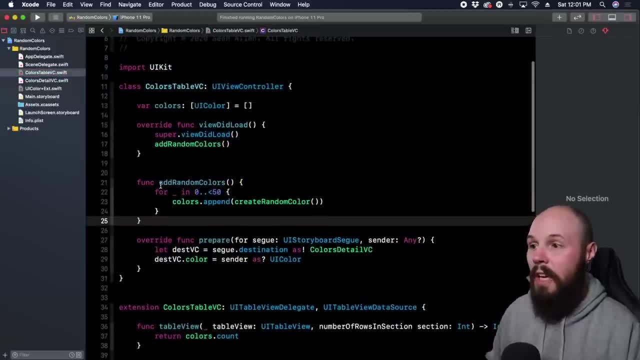 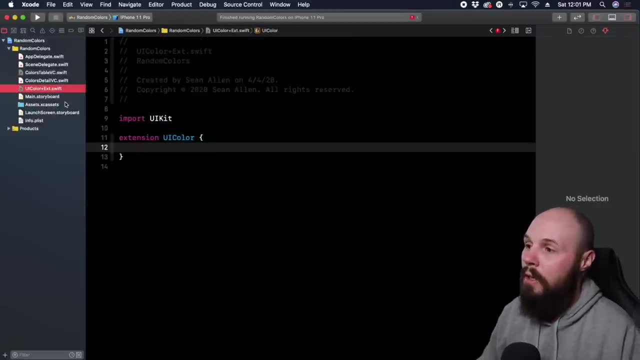 some changes. so command x space that out. so again, that cleans up our view controller. gets a lot of that code out of there. we'll come back to this error in a second. that'll be fixed. so go back to our color extension. now let's paste this in here. this needs to be a static funk, so every single ui. 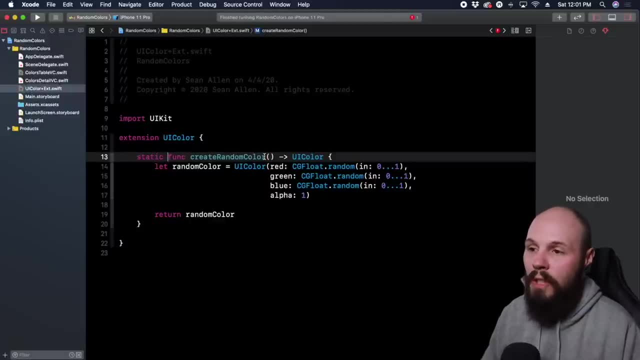 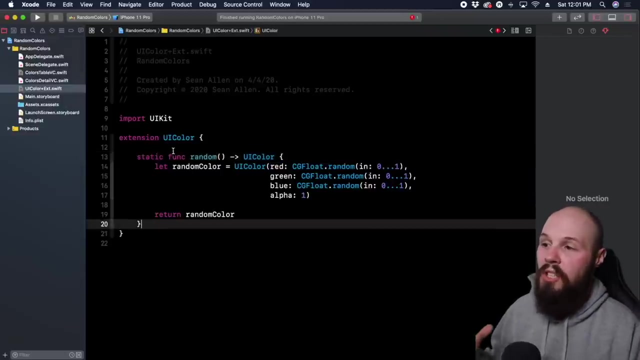 color has this, and then we don't want to say create random color. we can be a little bit more simple. we can just name it dot random. so when we use it we can just do uicolorrandom and that's it right. so clean, clean up some spacing here. so now we have a function on uicolor that will generate. 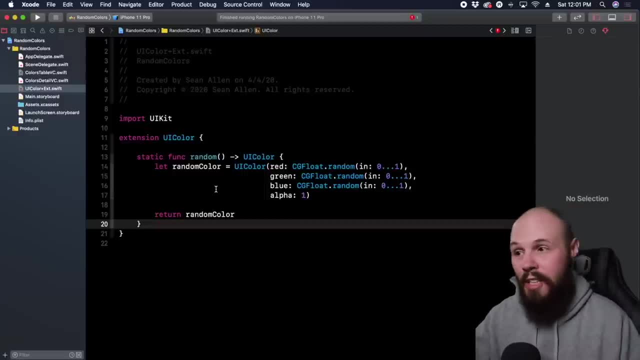 a random color. so all we did was literally just take that code, refactored it out into a uicolor extension by making it static. that means every instance of uicolor will get it, not a specific instance of it. so if we go to our colors table we see now that we don't have this, create random. 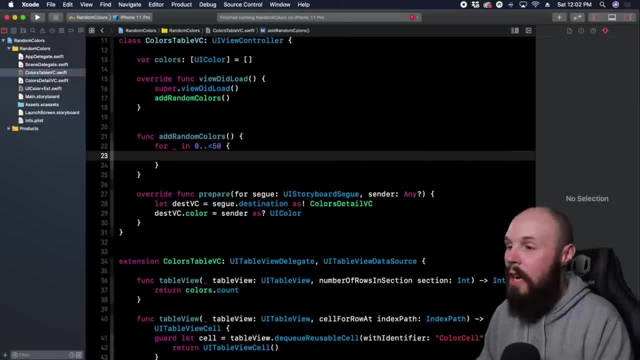 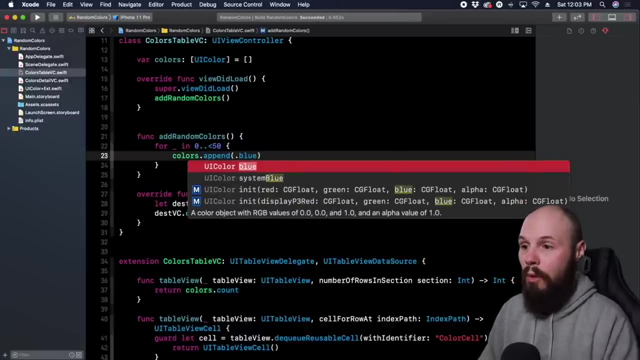 colors. i'm just going to rewrite this whole line so you can see what happens here. colors: dot append. and again for the type safety, right, it's expecting a ui color. so because it knows this is going to be a ui color, i can just do dot random again, just like i could have done dot blue or dot red. right, we're kind of adding a. 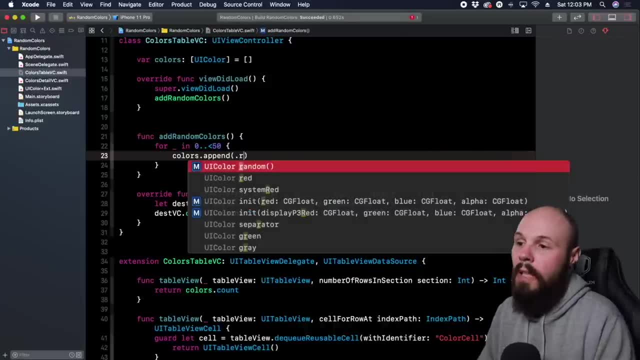 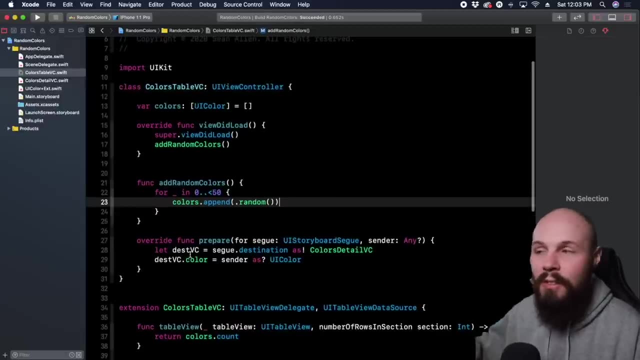 new color to our repertoire, except it's a random color, dot random. so there we go, colors, append, dot random. and again: now you see, we've cleaned up this view controller, we've refactored that code out into our uicolor extension, and again that spits out a random color here. so again a little. 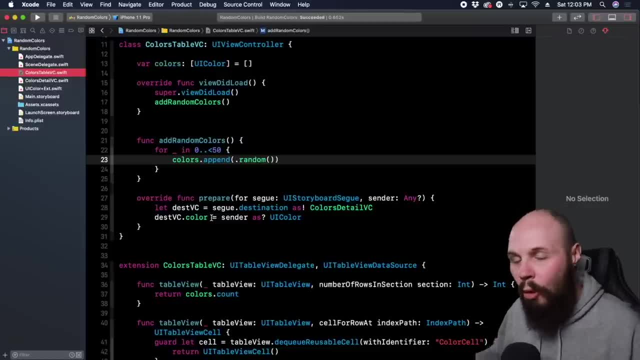 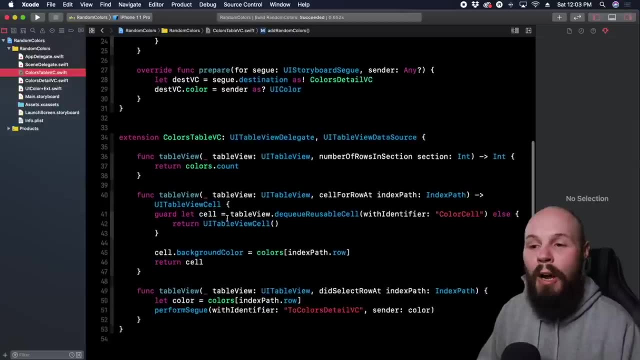 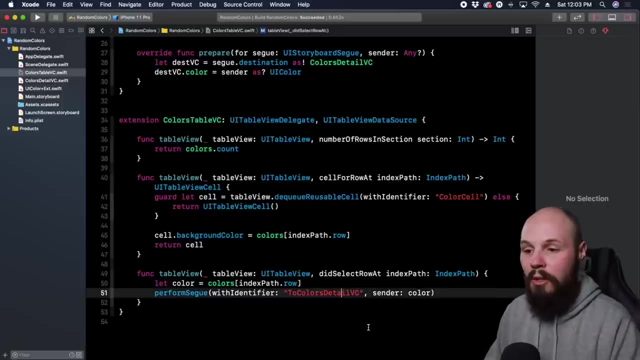 bit of refactoring. in the next video you're gonna see you know more refactoring, um, but uh, actually you know what? one more thing: refactoring is fun, i, i enjoy it. so back to remember how i said: these uh identifiers that are strings are a little bit dangerous because if you have a typo, you know if i just do two colors. 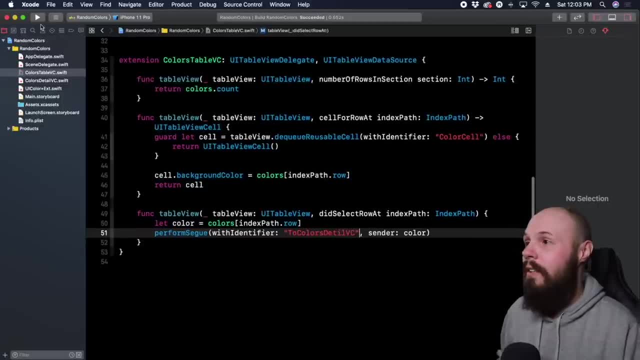 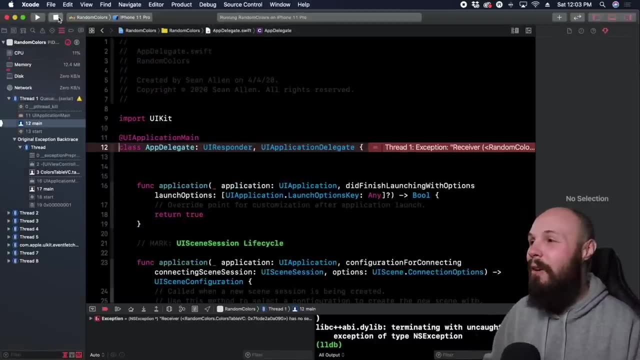 detail: vc. right, i just deleted that a. that's all right. now let's run it, just to show you. now, when i try to go to the next screen, bam, crash, right, something as little as that will crash your app. so i'm showing you here and i'm going to show you that it's not an official term, it's just a string. 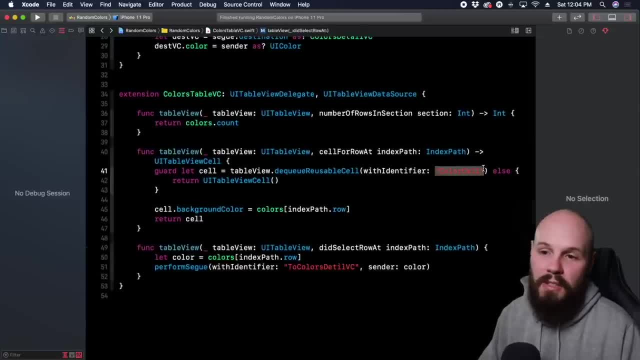 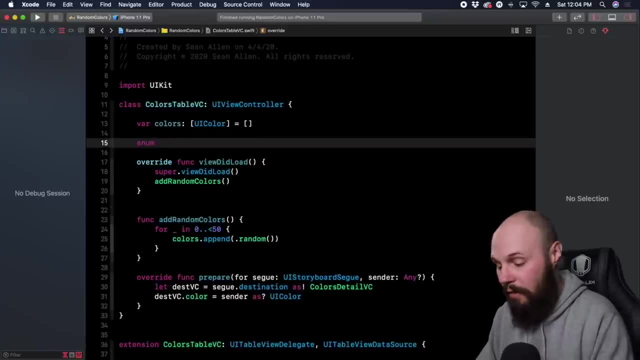 free of string already through the filter. that's what we're going to do, because we're not going to get to that unless we create an enum um. that's kind of like some slang. so on the left side right, it's just a string for stringly typed um. again, that's not a official term, it's kind of like some. 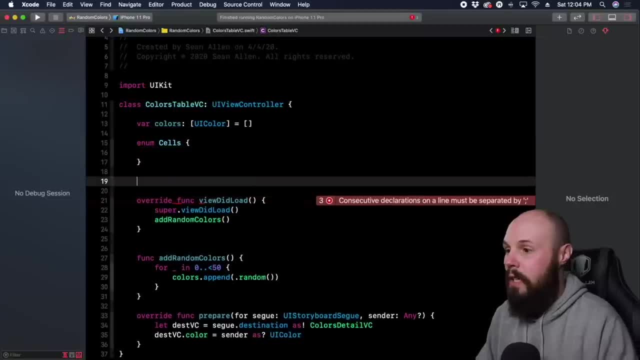 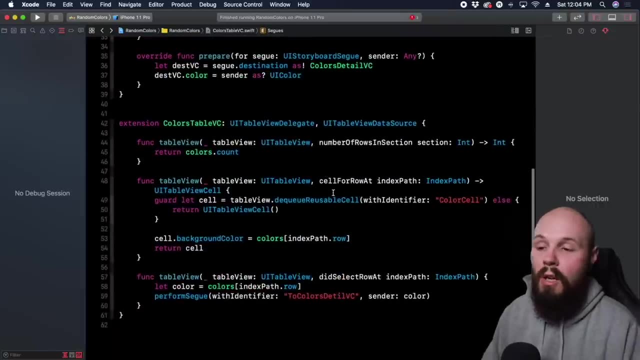 slang. so what we can do is we can create constants for these names, right, um, and you'll see here, what we can do is we can create an enum. so another purpose of an enum is to kind of have constants called uh cells, and we'll create another enum. 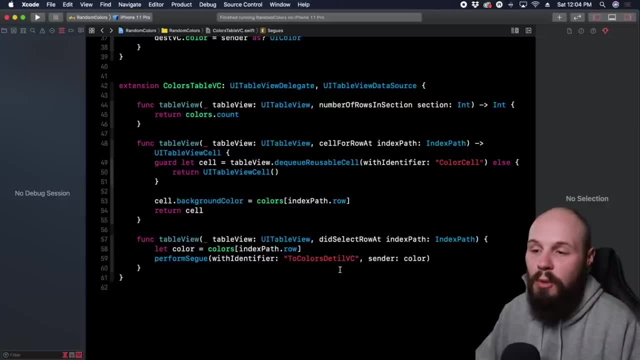 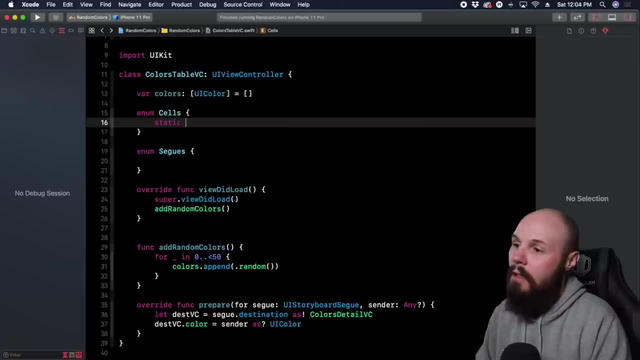 to a couple different screens, depending on the user's behavior. so you may have multiple segues. but what we can do here is we can create again a static- let call it color cell, equal color cell. so we're just kind of putting that string into a name and it may sound, it may look like. 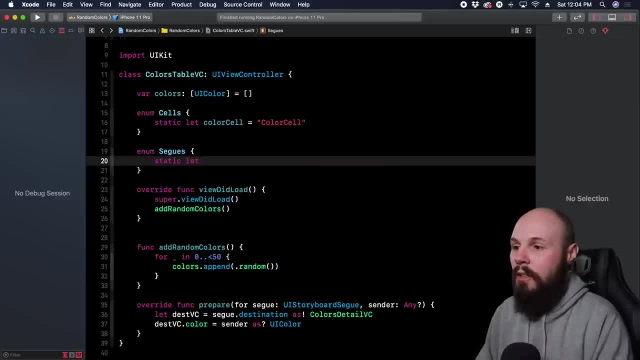 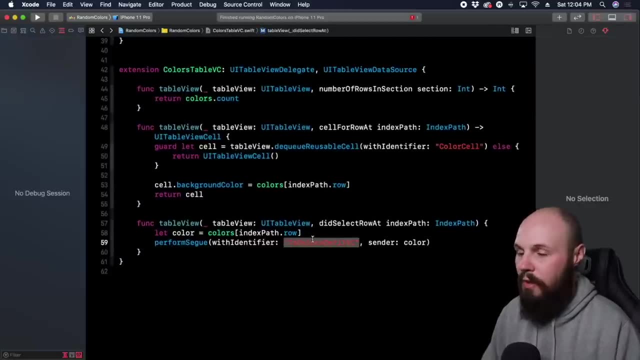 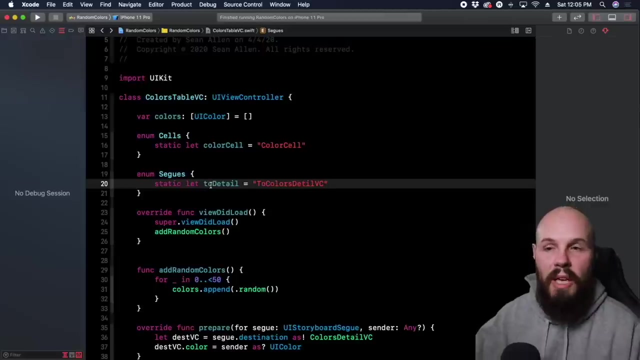 it's redundant, but you'll start to see the safety here. so static, let to detail, equal and we'll get this two detailed colors, vc right and you can name it whatever you like here. so you're going to see the safety here in a bit. so you define your segues, your cells, and again, it's not uncommon. 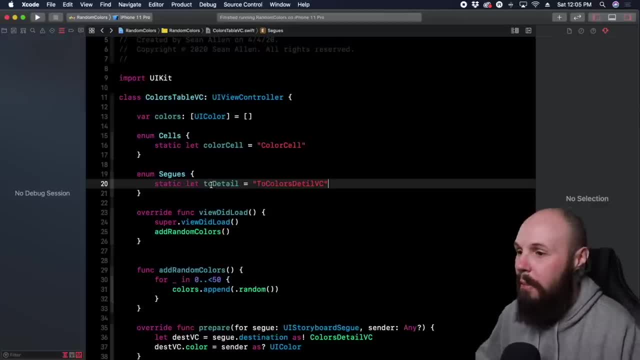 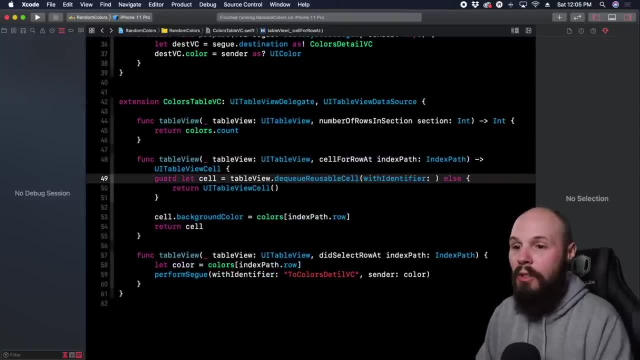 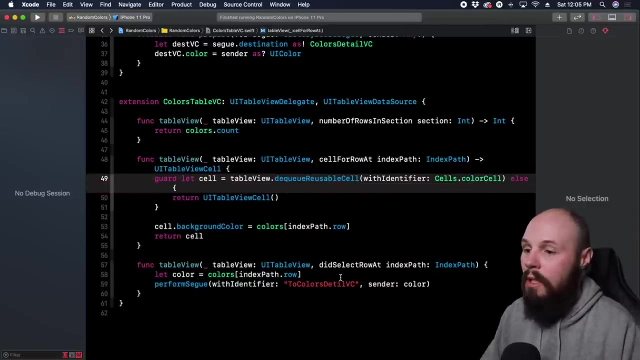 to have a screen with multiple segues and multiple different cells- not uncommon. so now, when i go to write in what identifier i want to use, instead of typing a string and risking a typo, i can do cells dot and you see, i get auto complete color cell. cells dot. color cell cool. 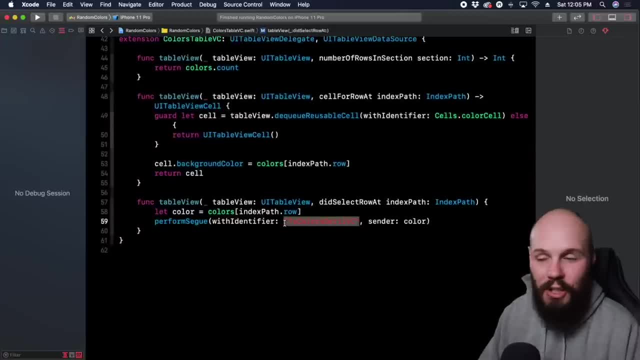 same thing here with segways. instead of, you know, typing in my strings for the segways, i can do segways dot to detail. so now you can see, you get the auto complete, you're not going to risk a typo and if you're using this color cell in, like multiple places, you don't have to type it out. 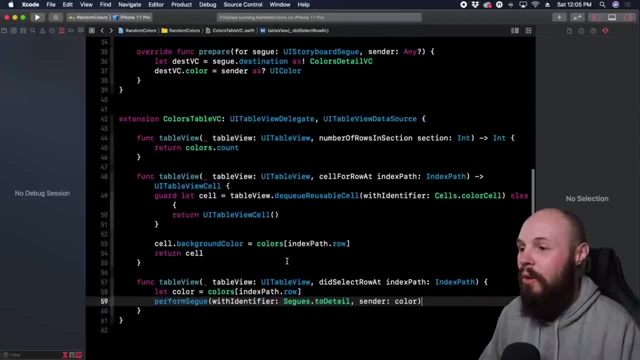 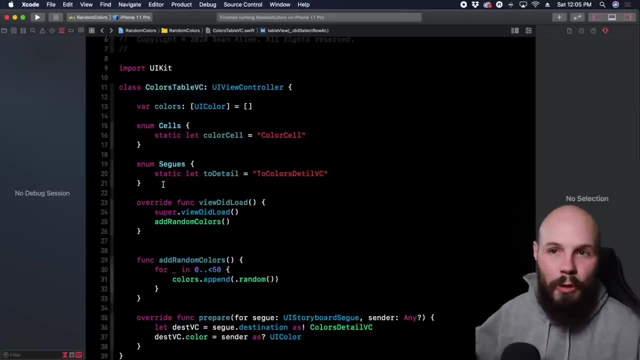 each time you got it in there in the constant um. so that's another nice little refactoring bit, uh, that i like to use. so, anyway, that wraps up this app. we're going to move on to our next app. we're going to build it first in storyboard and then you're going to get your first taste of no. 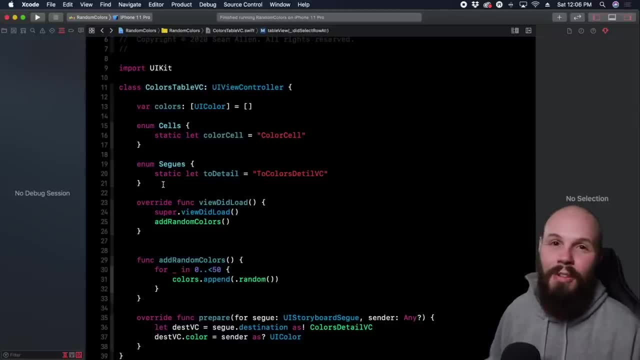 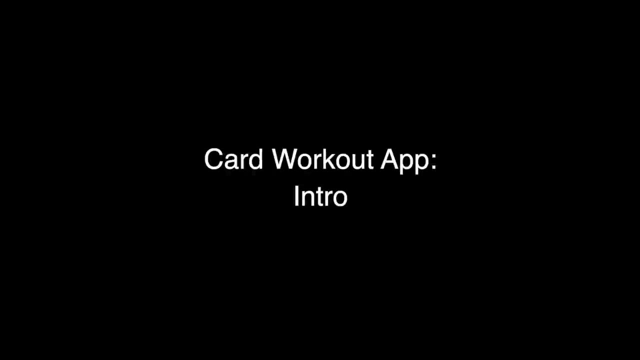 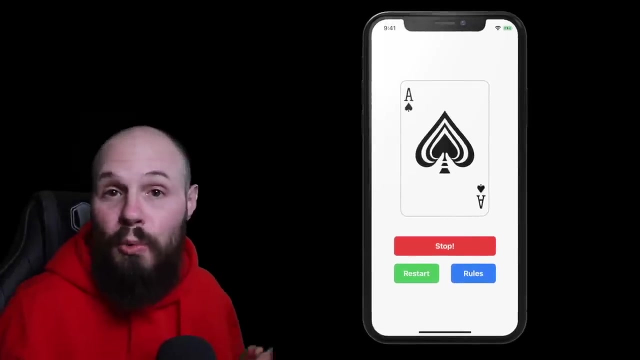 storyboard 100 programmatic ui should be fun. let's go. let's talk about what we're going to learn building this app. we're actually going to build this app two ways. the first way: we're going to use storyboard like we built the previous app, so this will be a little bit of you know review. 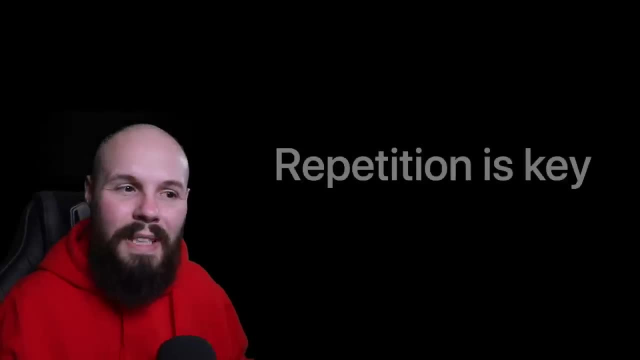 repetition. we're going to be building on our storyboard skills, but to me that's just key, right, like programming is just like anything else. you can't just watch one video or build one sample and then you know it. like, repetition and practice is the key. i mean, i know table views like the back of my hand. it's because i've built like. 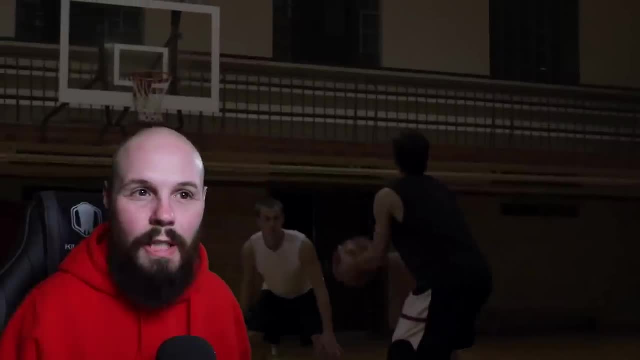 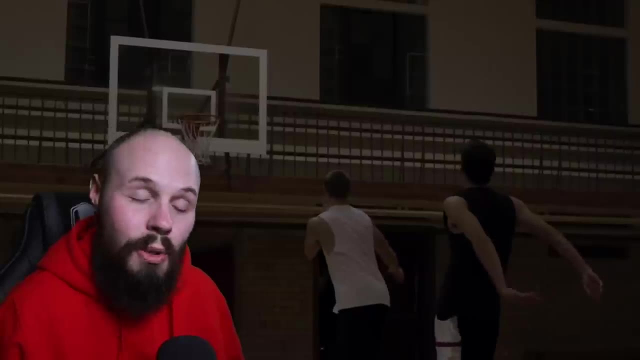 hundreds of them. right, and i like to compare it to basketball. right, if you're learning how to play basketball, you don't just go into the gym, shoot 10 jump shots and then go home and say, oh, i learned for today. no, you have to practice repetition. you have to be getting a thousand shots. 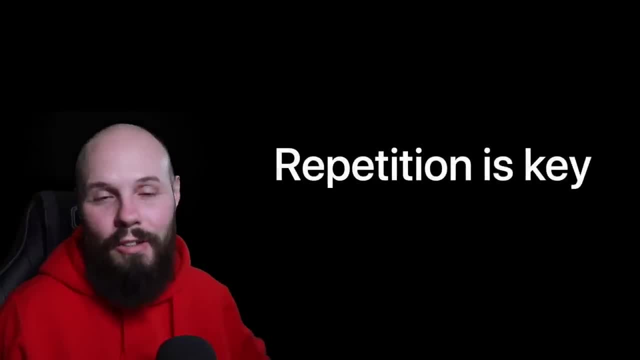 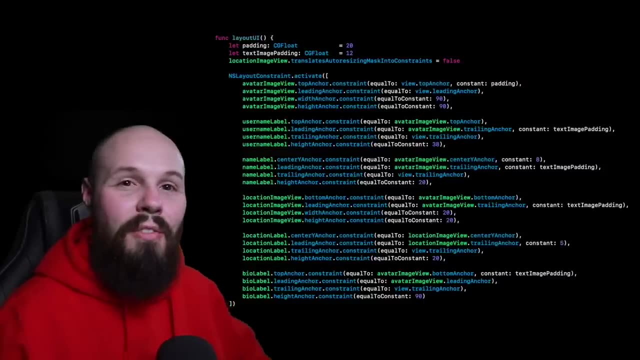 a day up, so repetition is a key thing. you've probably heard me go on that rant before, but there it was again. the second way we're going to build the app is the new hotness, the new stuff, and that is building it programmatically. i've touched on in a previous video. there's a kind of 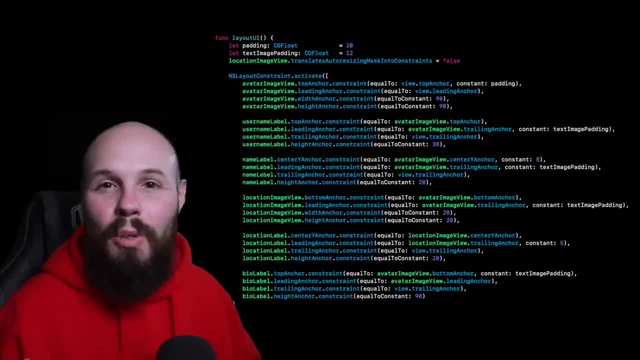 a debate storyboard versus programmatic. a lot of it comes down to preference, but there are some valuable pros and cons that we've already covered. however, in the next few videos, you're actually going to get to see first-hand programmatic ui and start to judge for yourself. all right, let's. 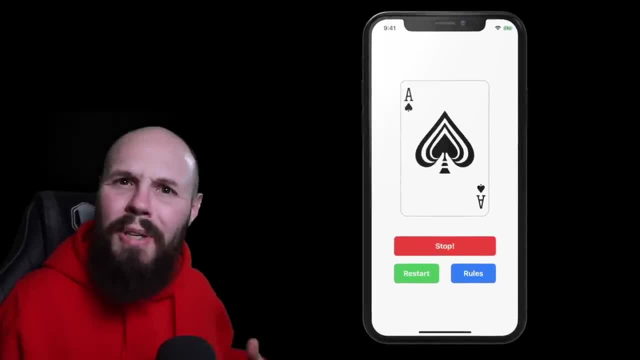 take a look at some of the pros and cons of this app. the first one is the functionality of this app, and the cool thing about this app is it's an app you could actually potentially use, and that's always a fun thing when you're you're legitimately using an app you've built. not sure if you've heard. 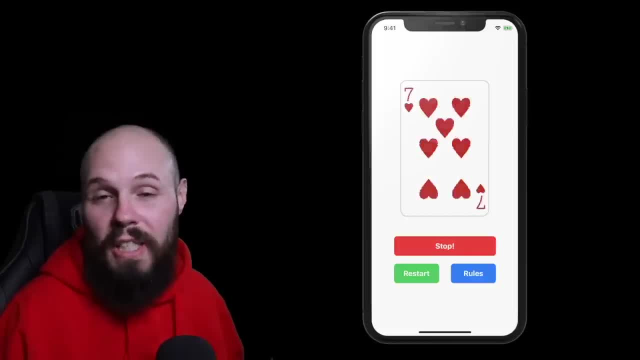 about, like some workout programs where they require a deck of cards, and then you pull that card and if it's, you know, the seven of hearts- and that means hearts equals push-ups- and then you do seven push-ups, right, and then you kind of cycle through the deck as you do your workout to give. 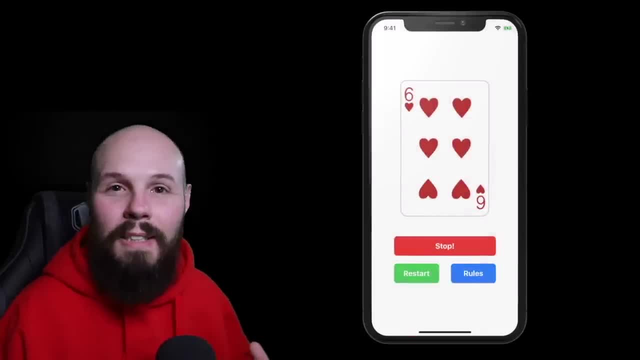 you some variety and in this example we're using, you know, push-ups, sit-ups, burpees, jumping jacks, but you can customize that to whatever you want to practice and use this app. so you kind of saw the functionality there. basically, this card image here cycles through a whole deck of cards at random and 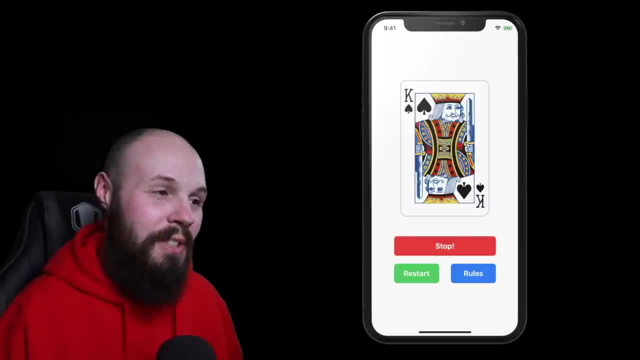 then you hit stop, kind of like you're you're playing a slot machine, right? you hit stop and whatever card shows is what you do on the exercise. and then you can hit restart to restart the timer and then when you tap rules, uh, the rule sheet will slide up. that'll show you. you know what equals. 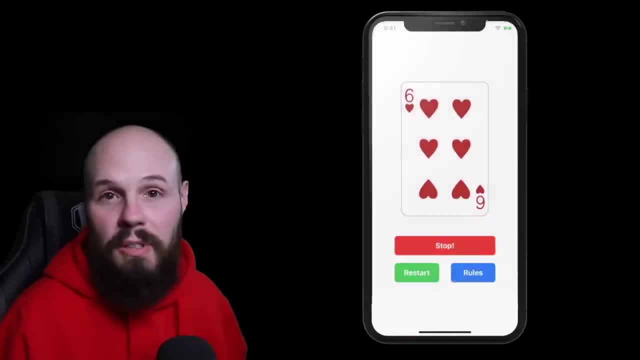 what right like a jack of hearts equals, uh, 11 sit-ups, you know, and then you can customize that and then you can click on your own settings and then you can set up your own custom settings. so again, it's kind of a little bit of a different approach to it, and then it's also, uh, it's a little. 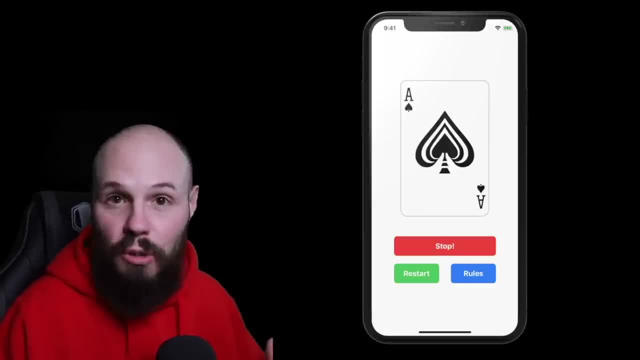 bit easier to do. so let's talk about the overall functionality. let's talk about what we're going to learn specifically. we're going to learn more about ib outlets and actions. um, the navigation right last app, we were in a navigation controller and you learned about that. this app we're going to 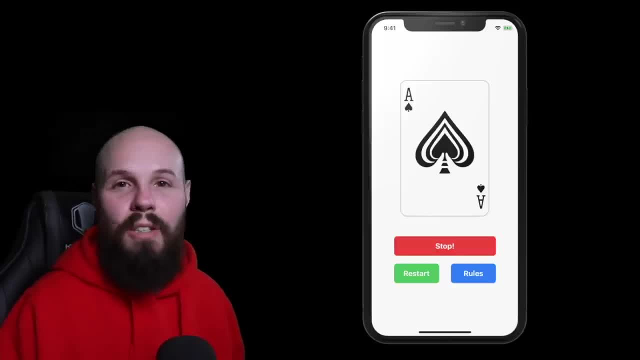 deal with those modal presentations that slide up from the bottom in more practice with the ui kit elements, you know, more buttons, ui image views, labels and again a little bit of refactoring. once board is going to be more review and building on existing skills. Programmatic: 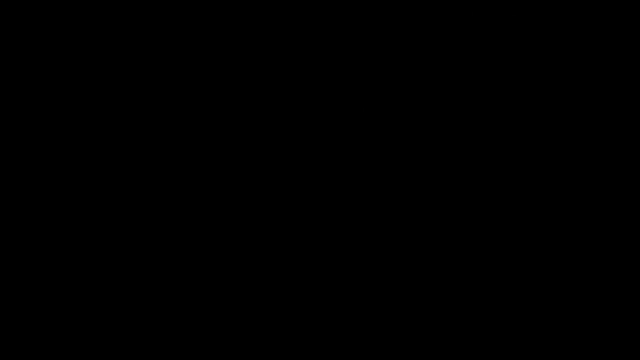 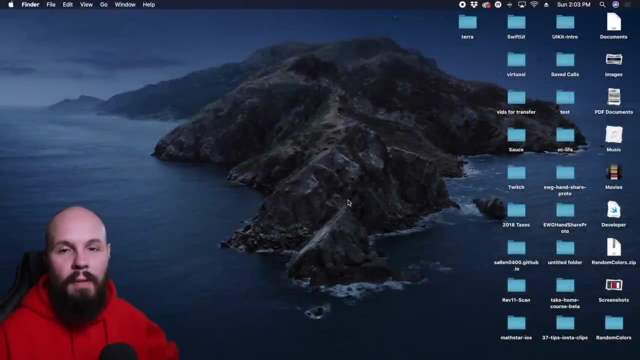 UI is going to be all new exposure, So let's get right into it. In this video, we're going to set up our project and lay out our UI on the story board. So, of course, come into your computer, create a new Xcode project. 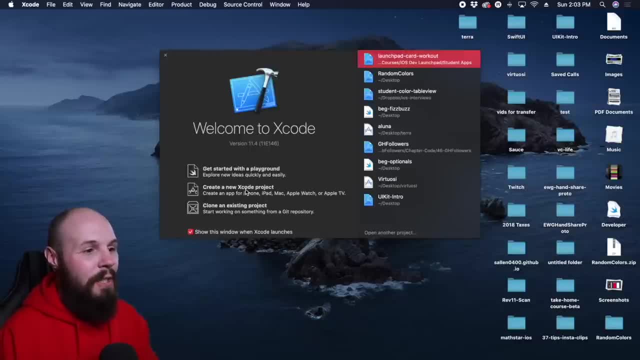 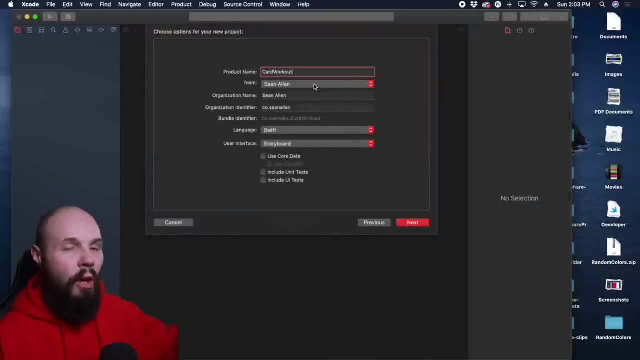 Hopefully you know you're getting pretty proficient at this. now Create a new Xcode project. single view application: hit next. I'm going to name this card workout and again it'll be all your team stuff, your information, Swift storyboard- hit next. 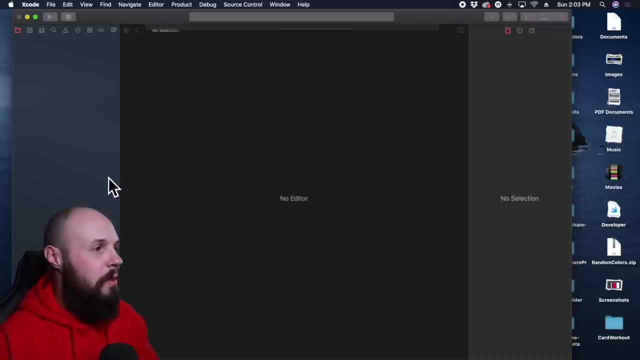 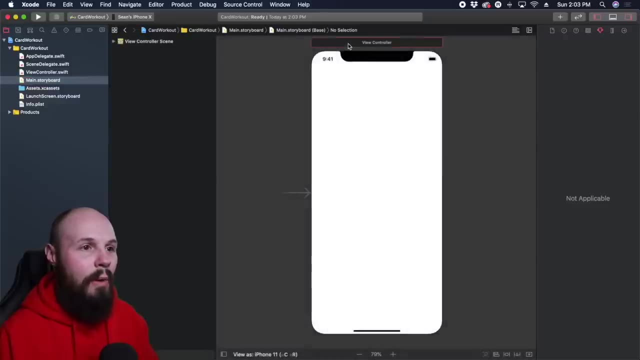 Again, I'm going to start moving a little quicker, because hopefully we've done this a few times by now. Should be a bit of a review. Alright, make my screen bigger. Click on our main storyboard and here we are. We have our view controller, So I'm 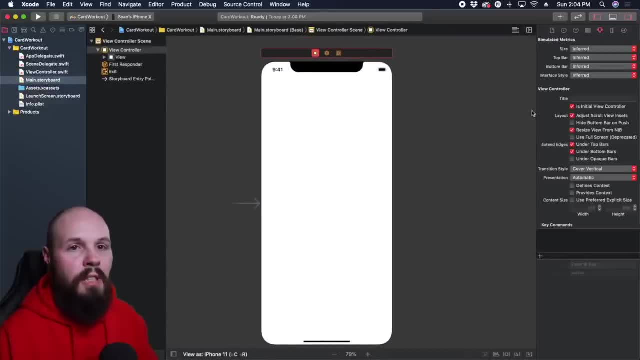 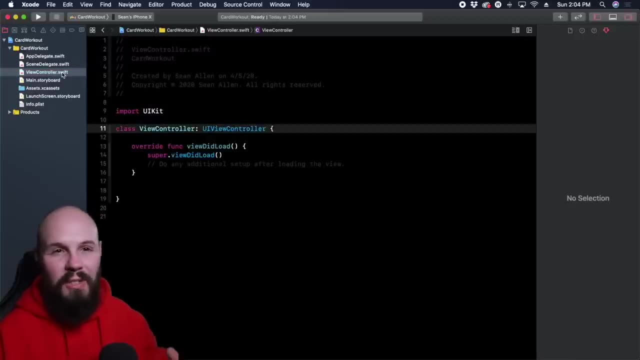 going to make some room here for my giant resolution screen. And there are ways to rename this view controller. right, because view controller is just a pretty generic name. But you got to be careful when you do that, because sometimes your file pathing will get messed up in Xcode. 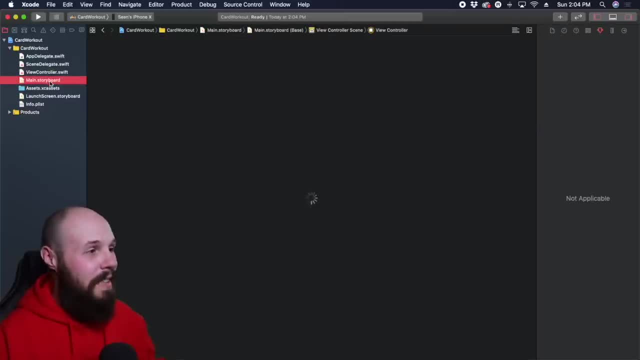 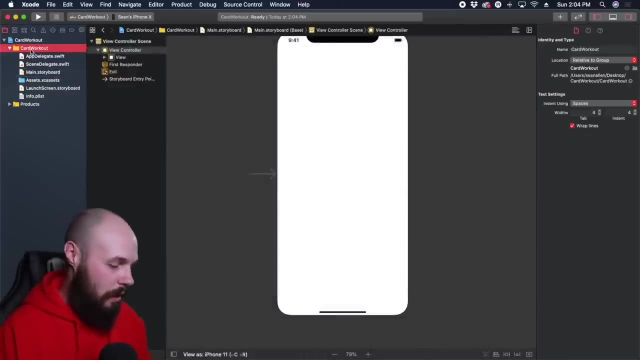 And again, there is a way to do it. I've just gotten in the habit of actually deleting that file. So right click on that view controller, hit delete, move to trash. that is gone. And then now I just do in my folder here: command N Cocoa Touch. 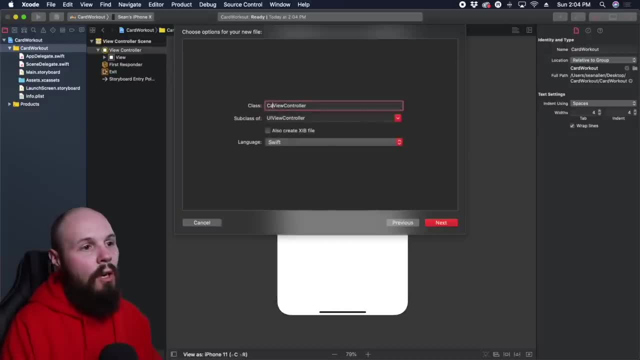 class next And then we'll call this card selection VC. right, And, like I said, there's a way to rename it. I'm sure somebody will chime in in the comments. I always just take the the 10 seconds it takes to create a new file. No big deal. 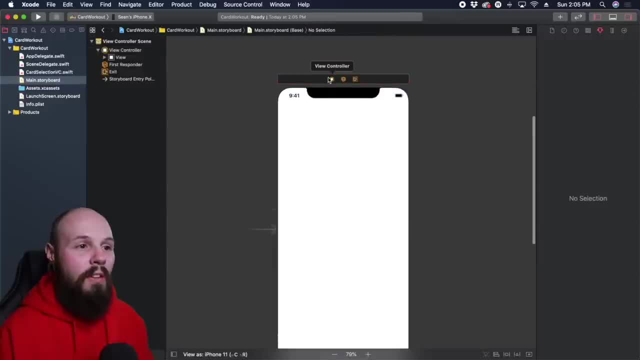 and there we go. So mainstoryboardcom Now, remember we have to connect this storyboard to that file. so you click on the view controller there, Hit the identity inspector. Instead of the class being view controller, make it a card selection VC. Alright, we're good to go. 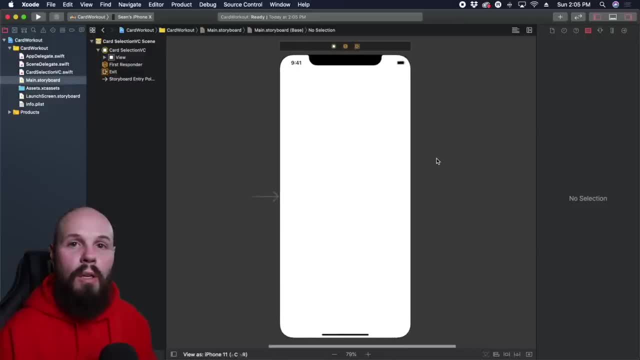 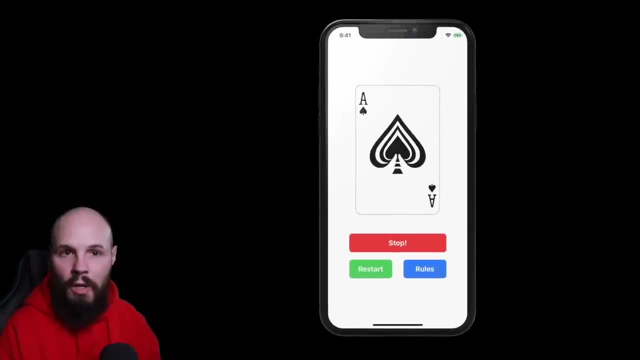 there We're renamed. Okay, now we want to start organizing our layout. so if you see on the screen here, see, we got a UI image view. that is a picture of the card and then we have three buttons below it, A relatively simple layout. So let's start by adding. 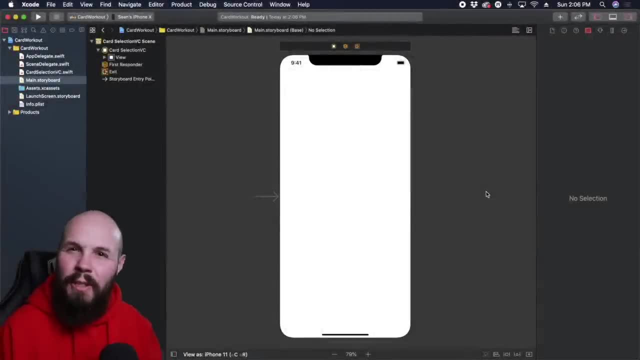 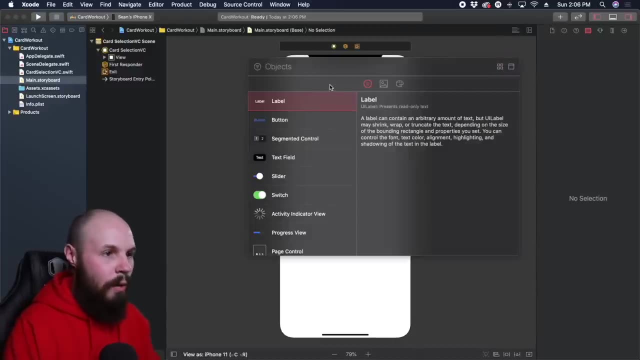 the big UI image view that holds the card. That's going to kind of be the anchor of our UI. we're gonna be pinning everything else to that, so let's do that. so hit the plus button here or again. command shift L. type: UI image view. so UI image view is. 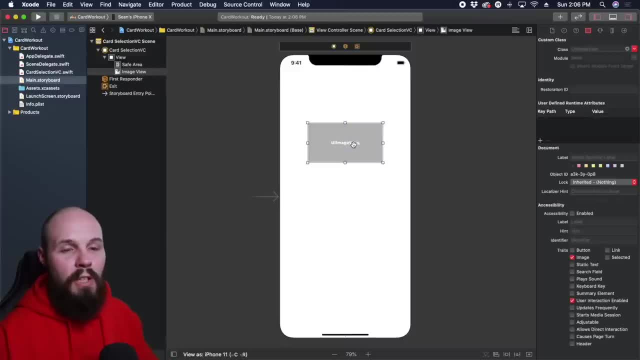 to hold the image, drag it onto the screen here now we want to constrain this. now a playing card is, I believe, like 3.5 inches by 2.5 inches, so to keep that math pretty easy on that conversion on the aspect ratio, let's hit the tie. 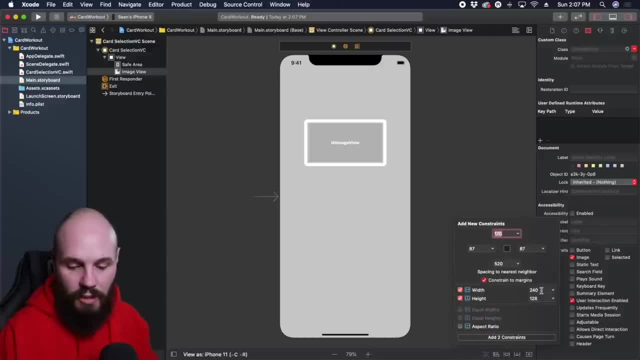 fighter here let's give a hard-coded width and height. so the width is 250, height is 350. so we get that nice card aspect ratio. connect those two constraints now in the alignment, one just to the left of the tie fighter we want to horizontally centering container and vertically centering container. so 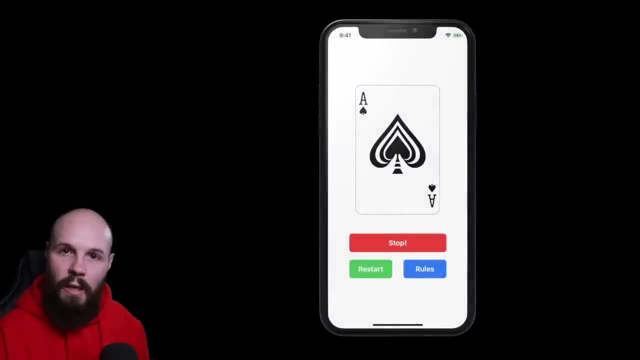 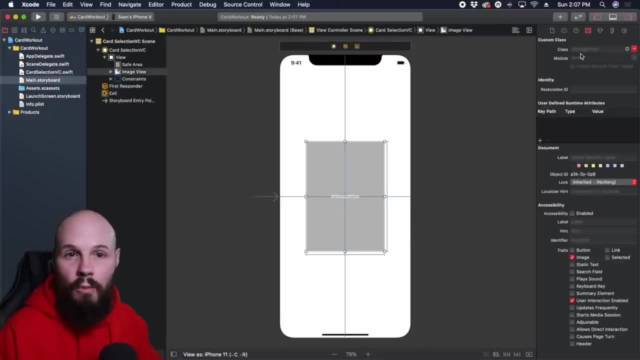 that puts the card right in the middle. but if you looked at our design, it shifted up a little bit. it's not dead center of the screen like this currently is. so if we click on our UI image view, go to the ruler, that which is called the. 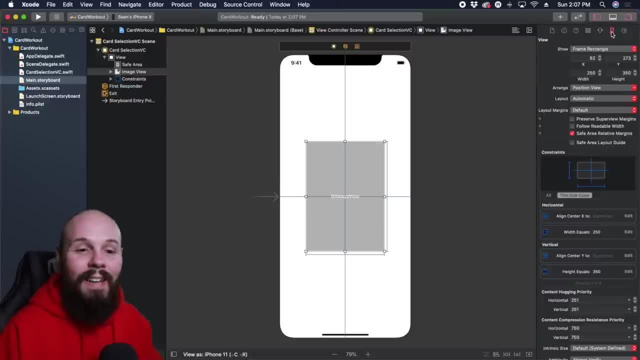 size inspector. I always just call it the ruler. and you see, we have our vertical image view and we're going to go to the size inspector and we're going to go to the size inspector. and we're going to go to the size inspector and we're going to. 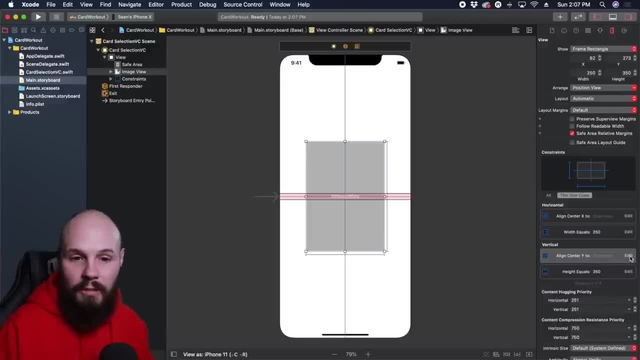 align center Y to super view. so click on the Edit button right next to that and now you can give it a constant. so we want to move it up, so we have to do like negative 100. so you hit that. now it slid it up 100 points from the center. so the 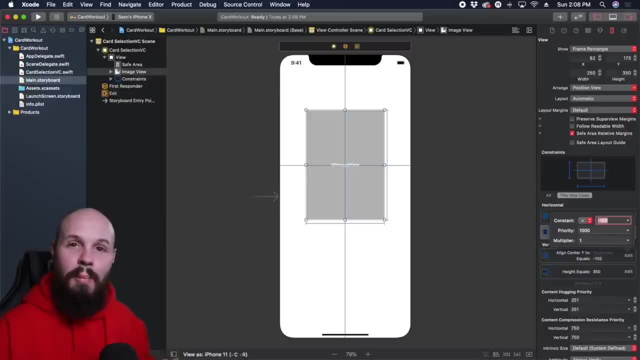 way that constraint works is it pins it to the center and then it slides it up 100 points. so that's how we're going to lay this out, and then we're gonna pin our buttons to the bottom of that UI image view and again back to auto layout. 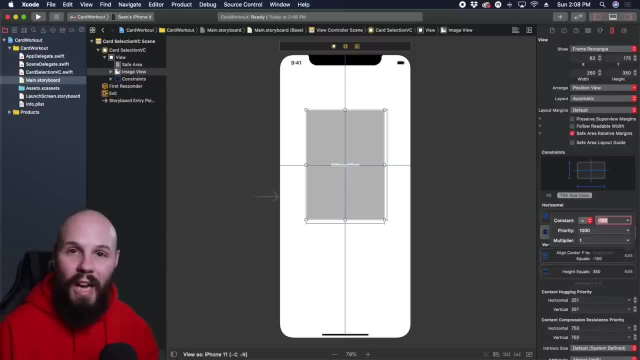 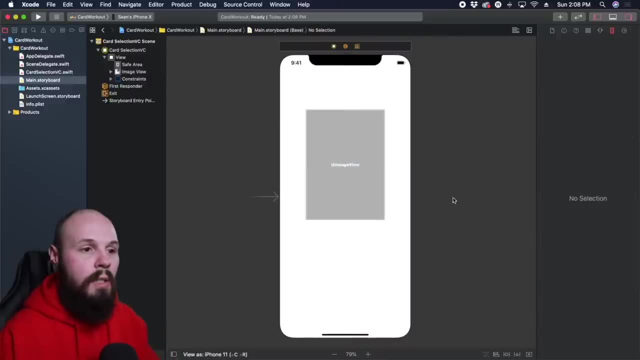 no matter if this is on a huge iPhone 11 Pro Max or the iPhone 5 or iPhone SE. you It's going to start it at the center and then slide it up 100 points, So make sure you hit return there to get that going. 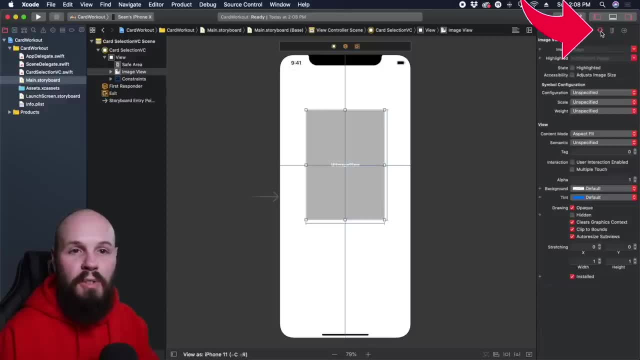 Click back on the UI image view Now in the attributes inspector. here we can set an image. You see right at the top, And now we don't have any images, right? What are we going to set that to? Let's actually bring in our assets, all those card images. 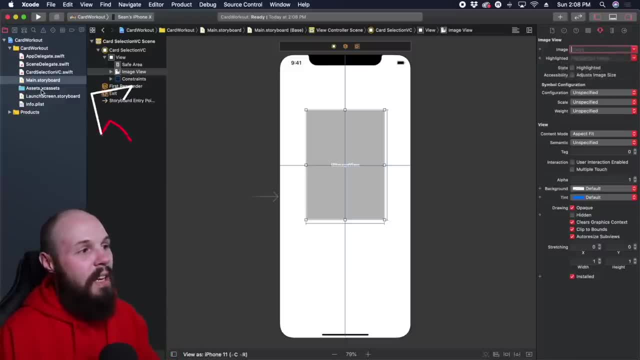 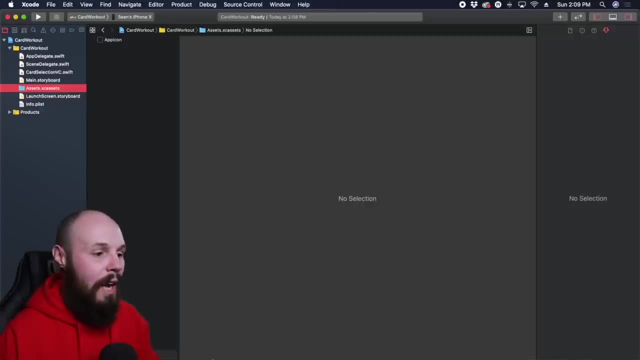 Now I have a file set up, but this assetsxcassets. this is where you drop images, So I'm going to attach a file to the description. It'll be a zip file that'll have all these card assets in here, but I already have it queued up and ready to go. 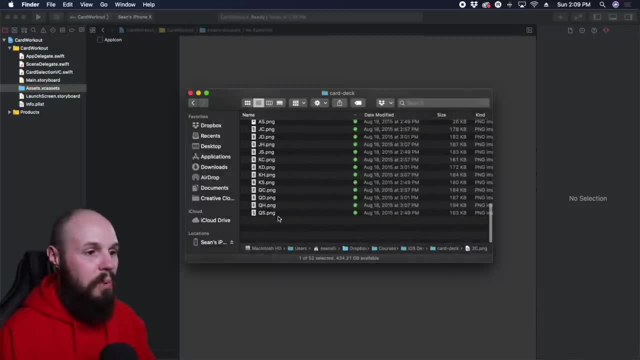 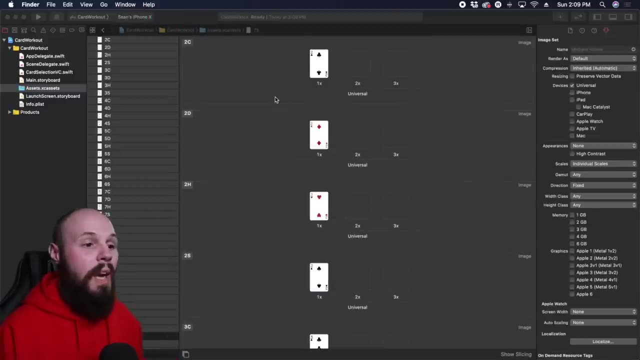 So here's like the two of clubs, two of diamonds, two of hearts, So I'm going to select all of these and drag it into my assets here. So this is how you bring in assets into your project. So now we have all of our card assets here. 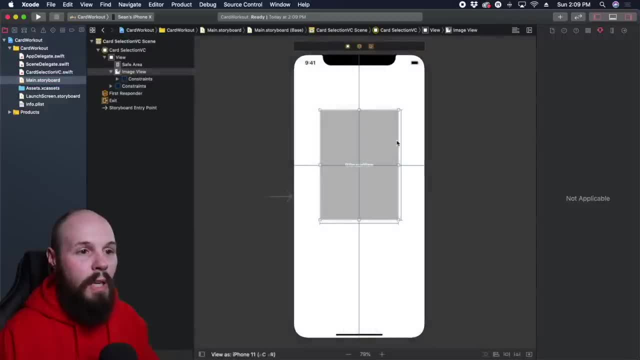 So back to the mainstoryboard. If I click on this UI image view now, when I go to image in this dropdown, you see we have all of the cards we just dragged in. So we're going to put- let's just put- the 10 of spades here. 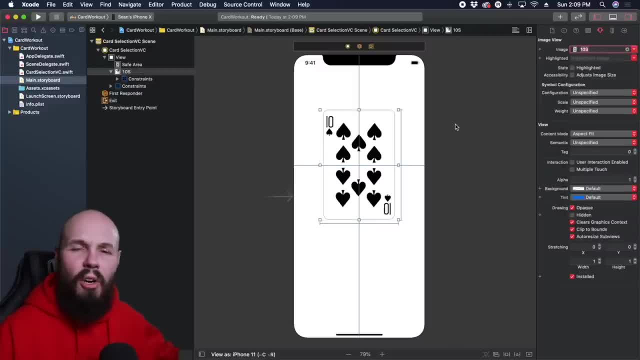 10 of spades Temporarily just to fill it. more on actually populating these cards in a later video, but we want to just get our layout showing up on the screen. So if you haven't picked up on it yet, the overall process of this video is going to be lay out- the UI. 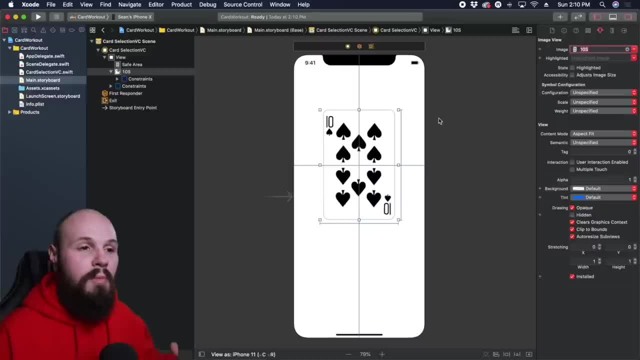 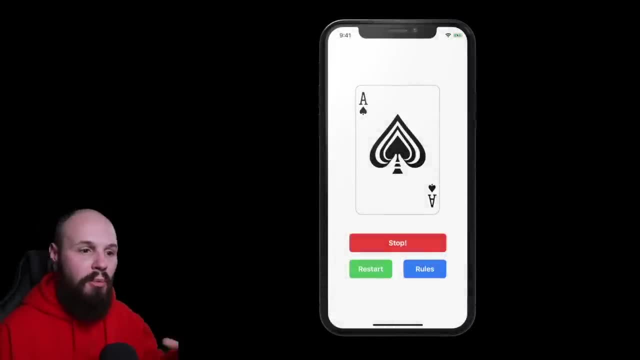 connect the UI and then write all the logic in the code to get the app running. So we're working on just laying out the UI right now. Now, pulling up our design again, you can see we have the card and then the three buttons below it, right? 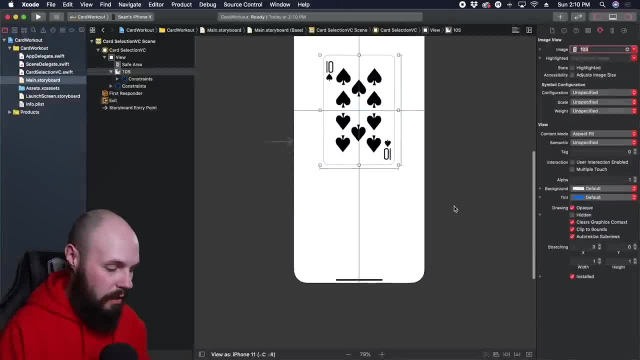 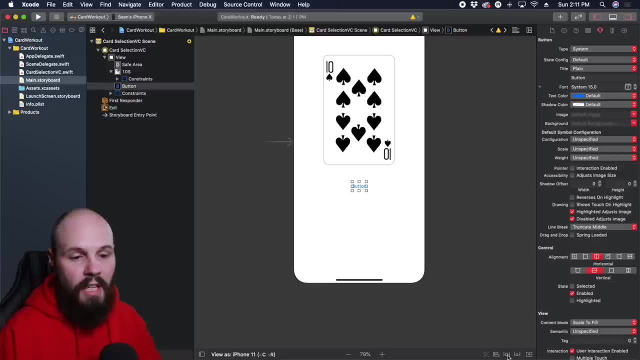 The stop, restart and rules buttons. So let's add those buttons Again. command shift L, Grab the button right here. There we go Now let's constrain this So down here in the TIE fighter, I want this width to be 260.. 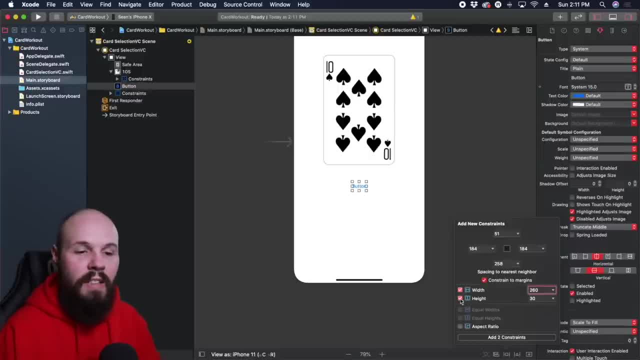 Again, this is just based on design choices. hard coding the width there. I like the height of my buttons to be 50.. According to the human interface guidelines, they must be at least 44 points tall and wide, because that's a big enough touch target for a human fingertip. 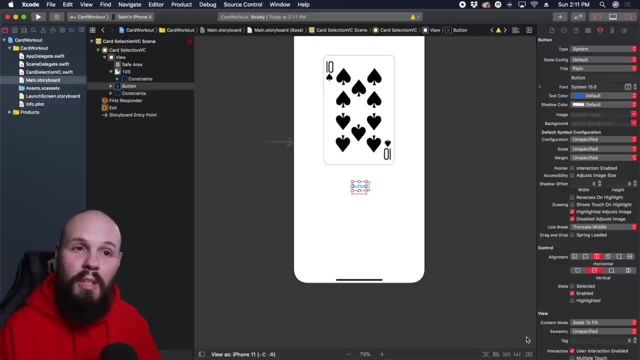 So if you're making buttons that are, you know, the width is less than 44 points or the height is less than 44 points, you're doing it wrong. So I like big, fat, meaty buttons, So I always go for 50.. 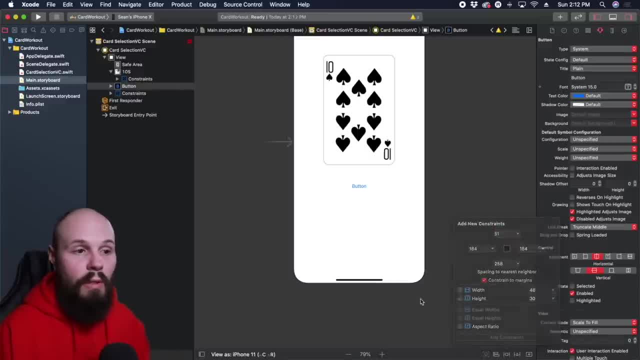 So now you can see, remember, when we're setting constraints, we need four of them. We only have two. We just have height and width, So we need to let it know where to be on the X coordinate. So here in the alignment tool, we're going to go horizontally: center and container. 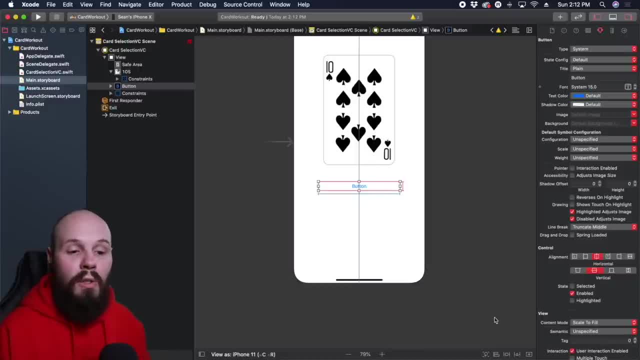 Cool, Add one constraint And then the last one is vertically right. So back on the TIE fighter, you can see the top constraint. We want to pin it to the bottom of the ten of spades. You can see here the UI image view, the little palm tree icon. 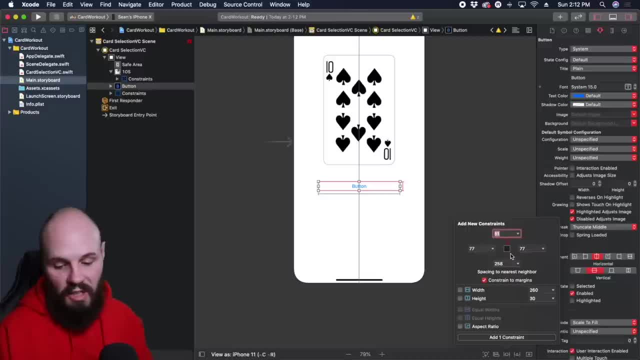 So if you click on that, we're going to get 51. Let's actually make this- I don't know- nice, even The number 60. So add one constraint And you can see it moved it down a little bit. 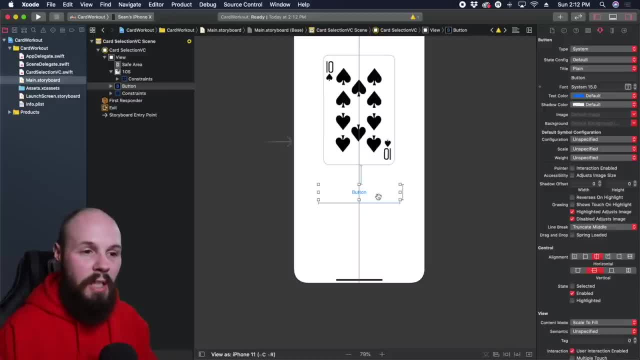 So we have our button positioned. Now let's style it a little bit here. So again on this button, you have the attributes inspector. We have the text color blue. Well, looking at our design, we want to make that white. 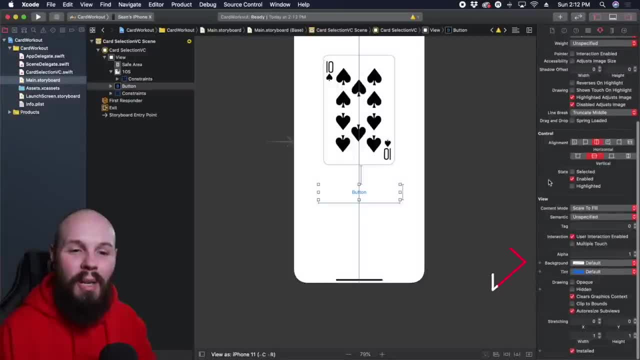 However, if we make it white right now, we're not going to be able to see it, So I like to set the background color first, which is down here. The background color is going to be the system red color. There you go. 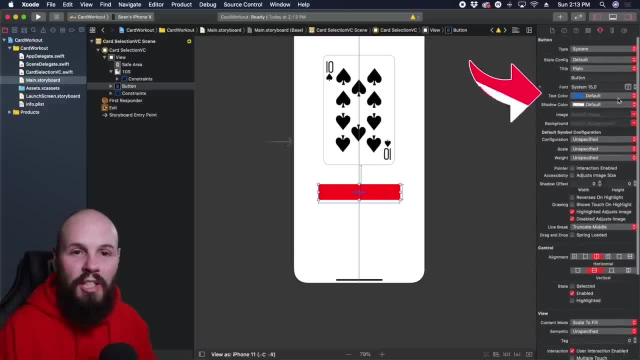 Okay, Now our button looks kind of. I'm sorry, our text looks pretty clashy, So we want to make the text color white. There you go. Now the words don't really stand out, So here we can change the font and the font weight. 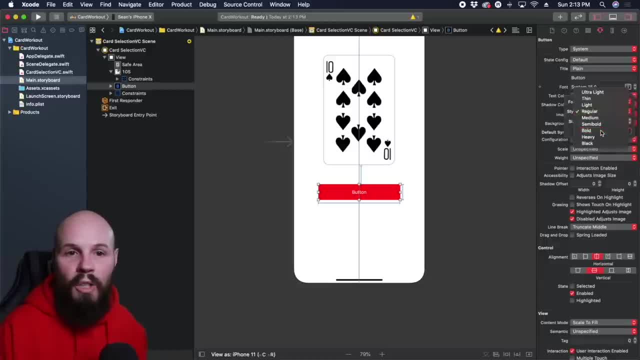 We're going to keep it system font. However, we're going to drop it to bold And we're going to make it like 19.. Again, big fat, meaty buttons that you can see, So you can play with fonts and sizes all you want, if you like to customize it yourself. 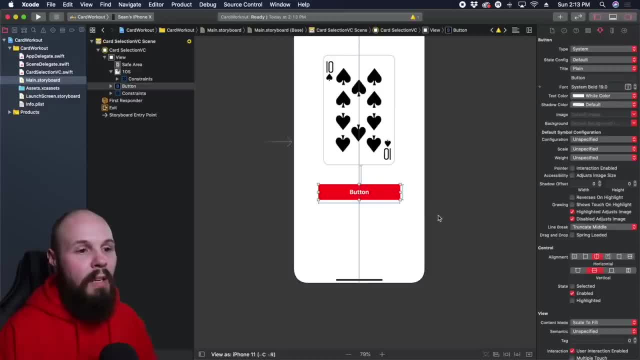 But that's what we're going to roll with right now. So here we have this button right, An easy way to kind of copy and paste buttons. That way you don't have to go reformat that again If you hold option. 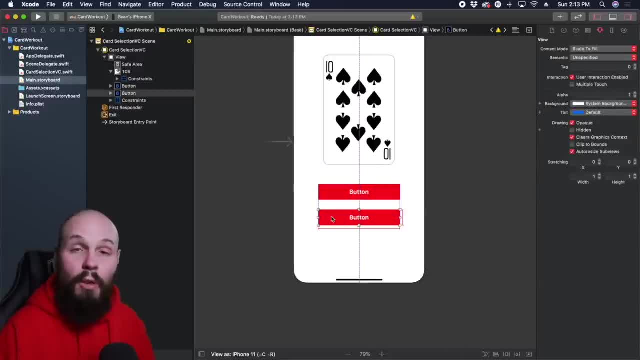 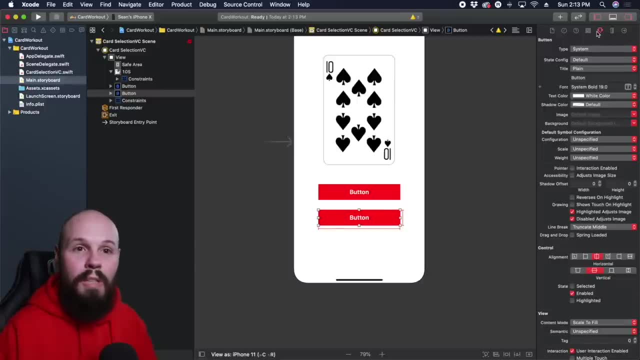 And then click and drag down on the button. Now, here you go And then let go of the mouse button first before you let go of option. Trust me, that'll get annoying for you. Here we can make a second button. So now we're still in the attributes. inspector of this button. 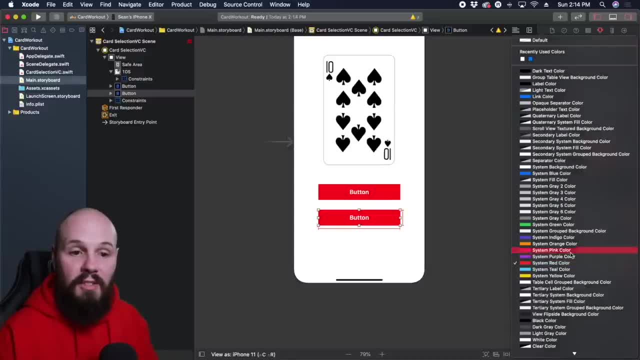 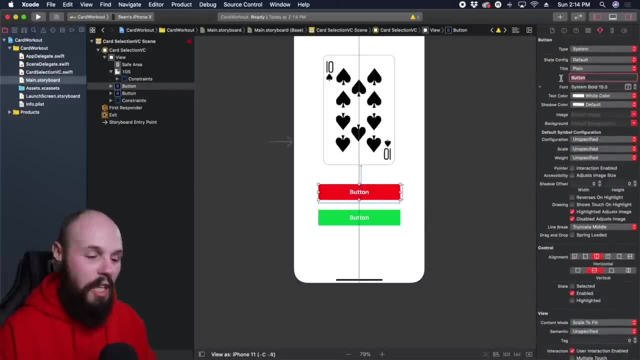 Now we want to make this background a different color, System green color, And we want to. we forgot to do this on the red button too, So go back to click on the red button. We want to change this wording here in the title to stop. 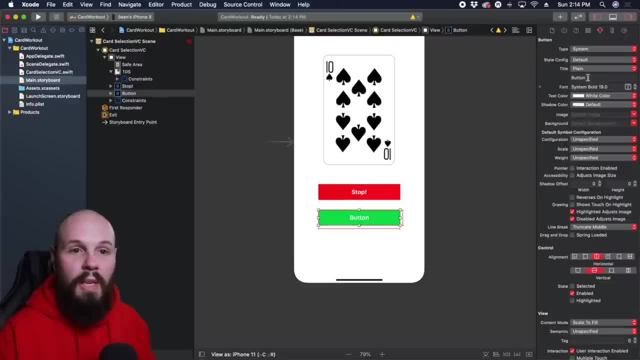 There you go And then click back on the green button. We want to make this title instead of button. We want it to be restart. Okay, now you'll notice we have red constraints here. That means we haven't fully constrained it. 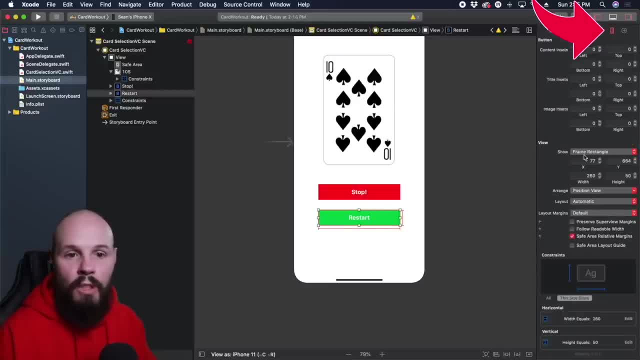 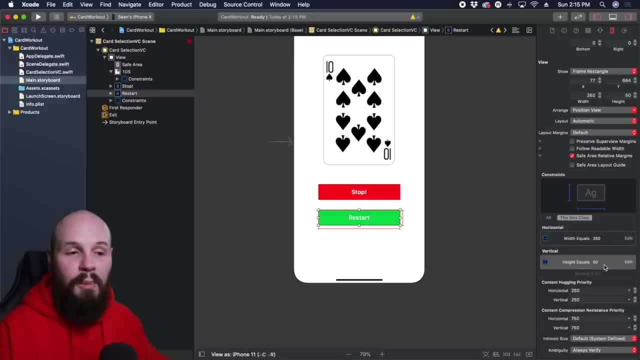 And we can double check that by again clicking on that button, Clicking on the ruler, scrolling down. You see, we just have a height and width And that's what carried over when we kind of copied and pasted it or duplicated it by holding option. 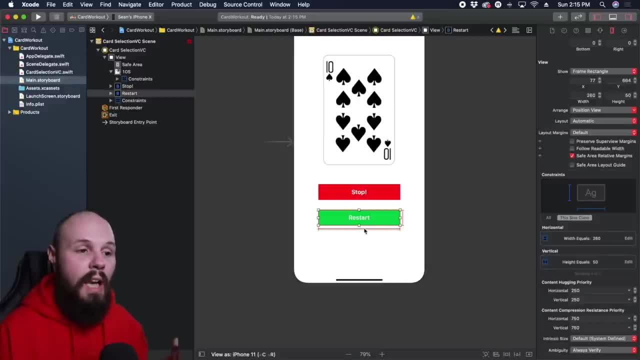 It'll bring over the height and width that we set. So again now we just need to give it the x and y coordinates. However, again back to the design, We don't want this to be the same width. I mean, you kind of want it to be the same width. 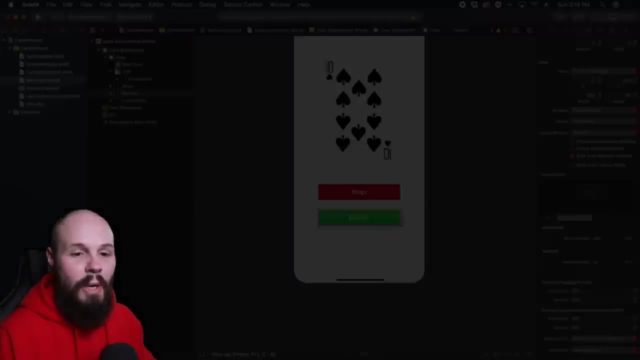 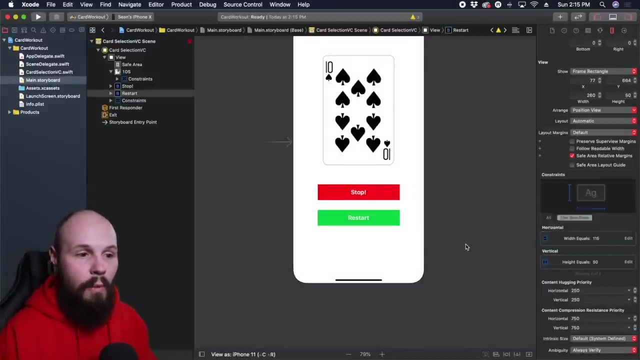 You could do three buttons top to bottom if you like. That's not the design choice I went with. So we want this width to be edit 115.. I'll tell you why here. So hit return And that will make this 115 as soon as we set the other constraints. 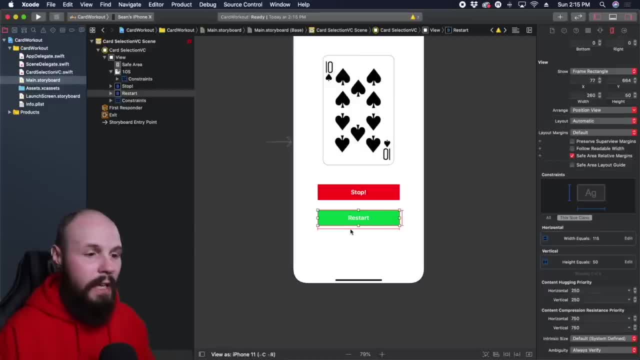 It'll do that, So let's do that real quick. Here's what we can do. We can hold, control and drag, And I'm showing you multiple different ways to set constraints to this object. And what we want to do is we want vertical spacing of that. 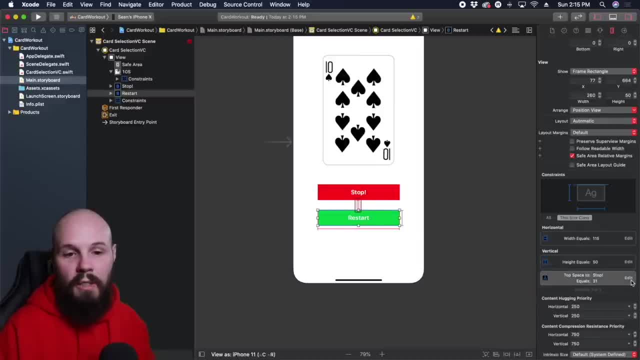 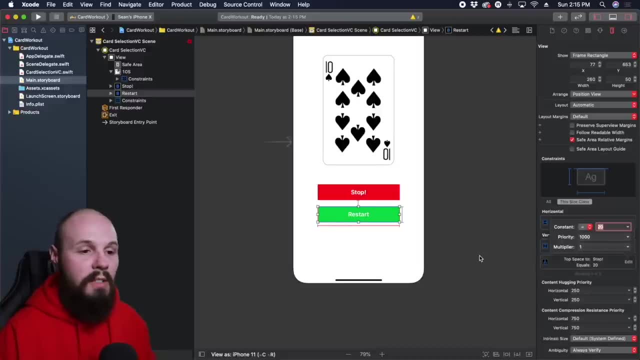 And you can see over here now, top space equals 31.. You see it down here. Well, now we can edit that, And I want 20 spacing in between, So you can set the constraint and then go ahead and edit the constant. 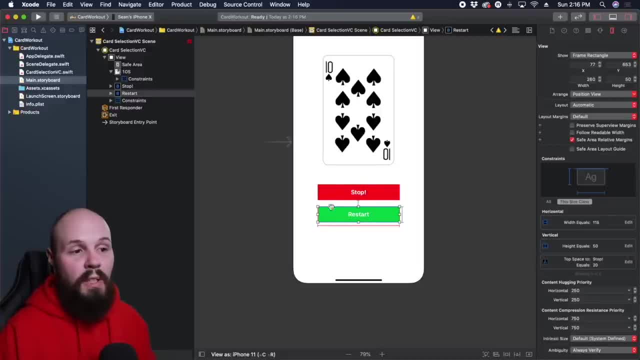 So now we need to know where it is horizontally Like we centered this one. However, for this button- again looking at the design- we just want it to line up with the left side of the red button. So if you again control, drag up to the red button, let go. 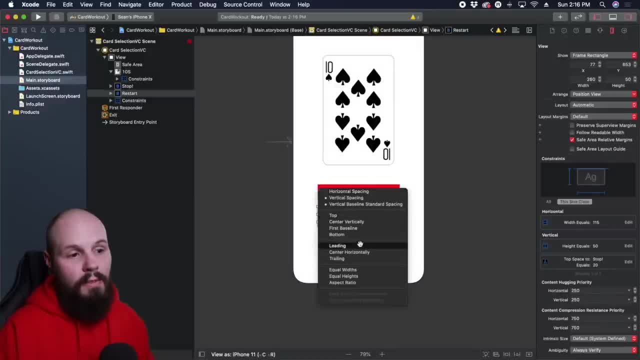 Now you can align leading. You see that here That's going to align their leading, which is the left. So leading is the left, Trailing is the right If you're in a left to right language, if you're in Arabic, and it's right to left language. 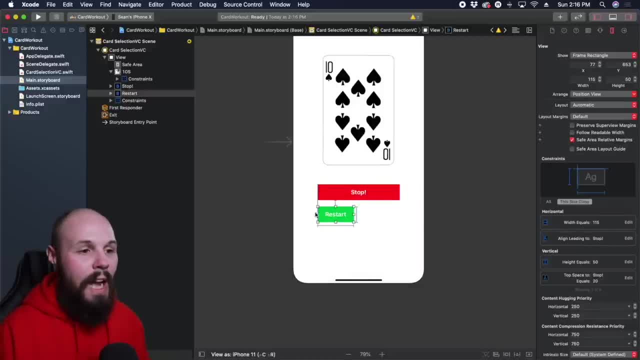 those are flipped, just so you know why it's leading and trailing. So now that's going to line those up to the left. And you see, when I set the fourth constraint it gave me that size of 115.. I'm sorry, the width of 115.. 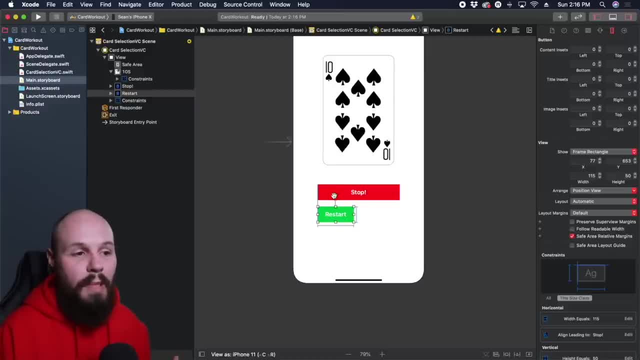 And the reason we did a width of 115 is because we wanted to line up nicely. This red button is 260.. So if I make this 115 and the other button 115, that'll give us a nice spacing in between. I didn't want to just divide 260 by 2. 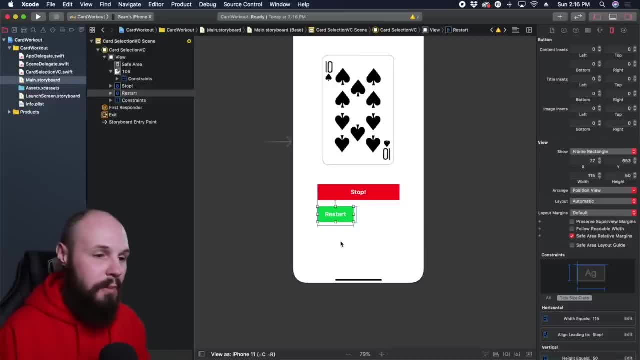 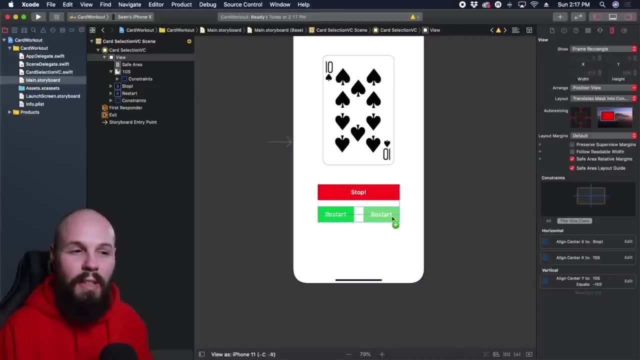 because then these two bottom buttons would be touching, There'd be no spacing, There'd be no space in between them. So, speaking of that other bottom button hold option, drag now to the right And you see, Xcode will kind of snap to it and line it up for you. 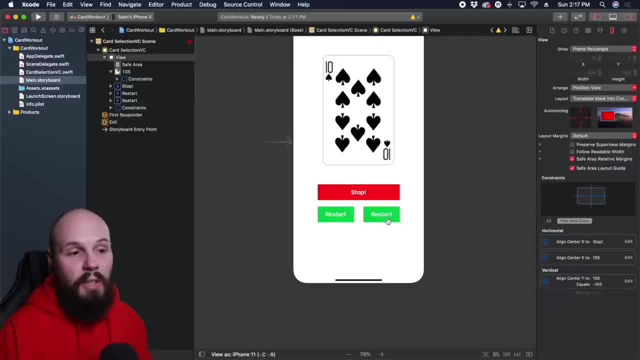 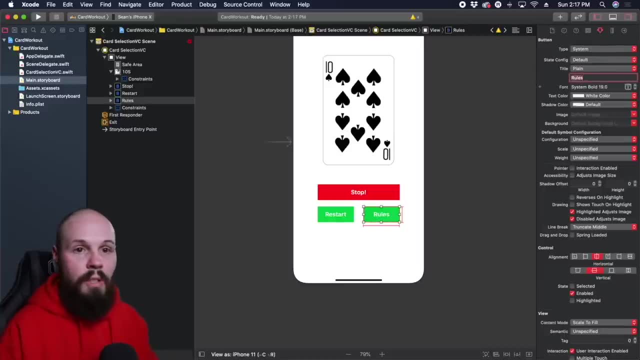 That's a nice little feature here. So now we're on this green restart button here, which is going to be our rules button. Okay, back to the attributes inspector. Instead of restart, we want this to say: rules, Hit, return And then the color instead of green. 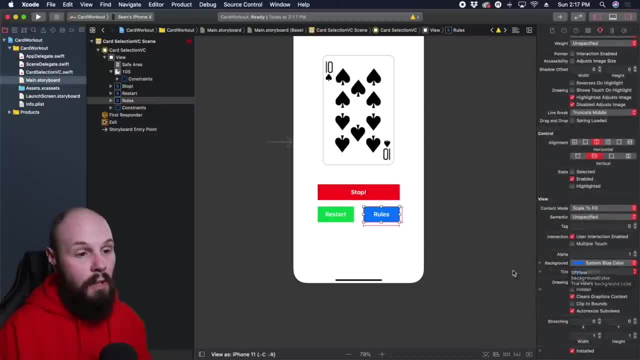 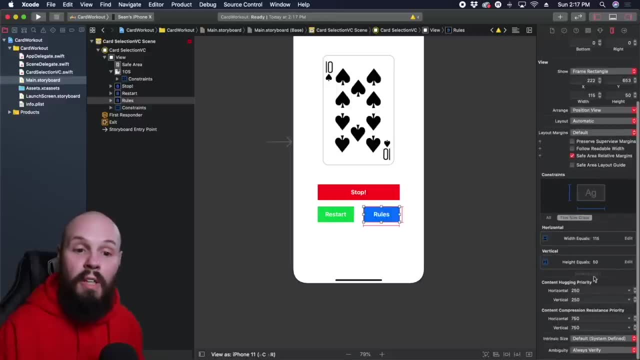 we want this to be system blue color. So there you go. We're missing some constraints. now Again back to the ruler button. on the blue button You can see we have our 115 width and our 50 height. That's two out of the four constraints we need. 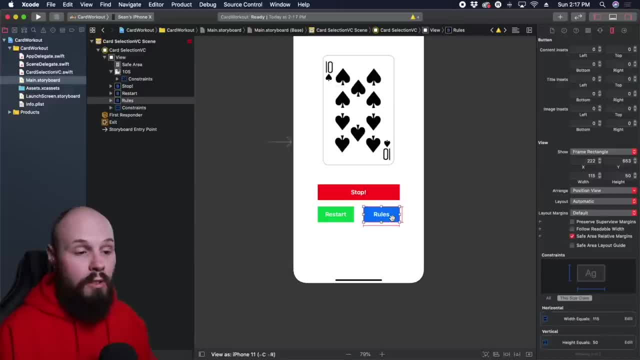 So we can do this two ways, if you really wanted to, Just like we did with the green button, we can set a vertical space to the stop to let it know where to be horizontally, or we can pin it to the green button and center vertically. 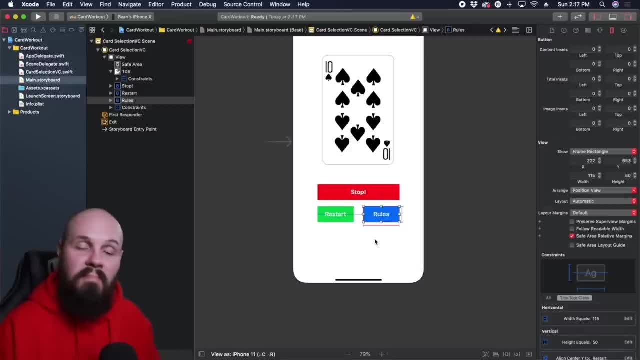 So now it'll be centered vertically with the green button. Both ways are fine. Again, whatever way you want to do it. So now we need to know where to be. again, horizontally, So same thing. You could set a specific distance. 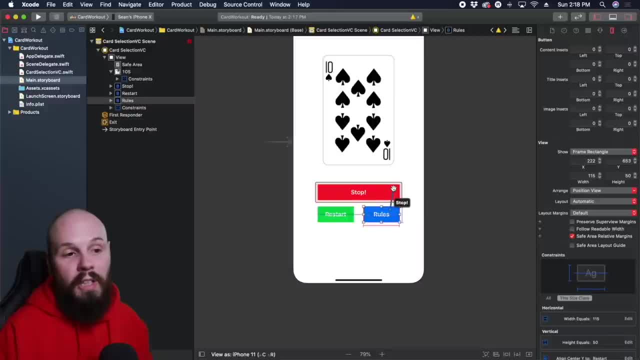 between the blue and the green, or you could align the trailing with the red. So again, there's a lot of options when it comes to how to constrain your layouts, But here we're going to go trailing so that way it lines up with the right side of the red button. 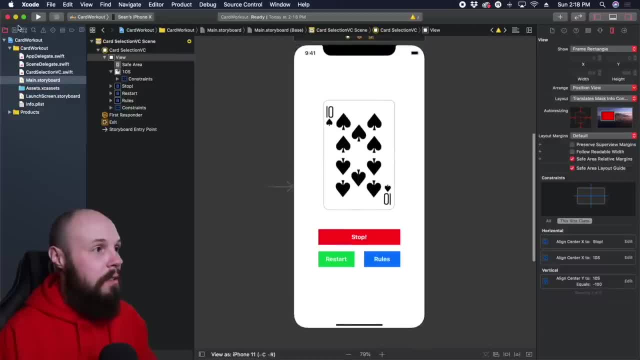 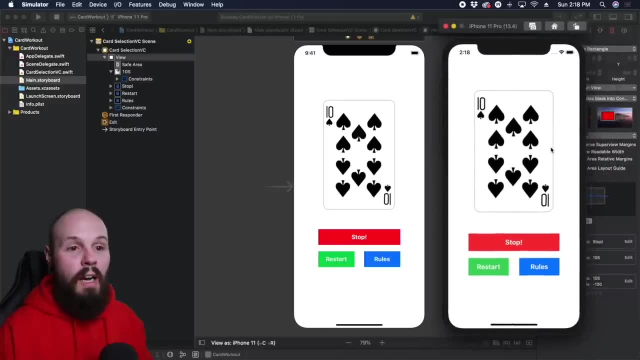 So now our app is constrained here. Let's run it and see what we got. iPhone 11 Pro Running it. And here we are. You see the simulator on the right. Put it side by side Looking good. Let's test it real quick on the iPhone SE. 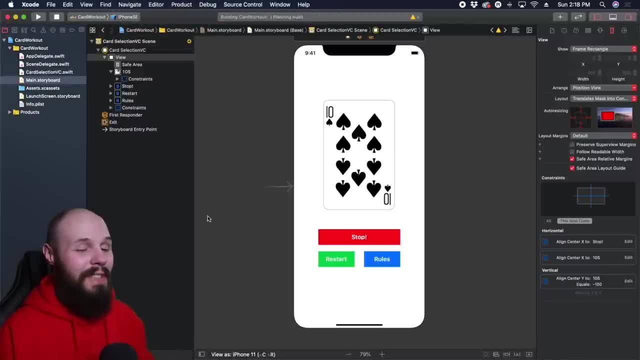 And I'm not going to lie to you, I have not tested it on the iPhone SE yet, So it should be fine. But if it's not fine, we'll see. So here's the iPhone SE. We'll put it right here on this side. 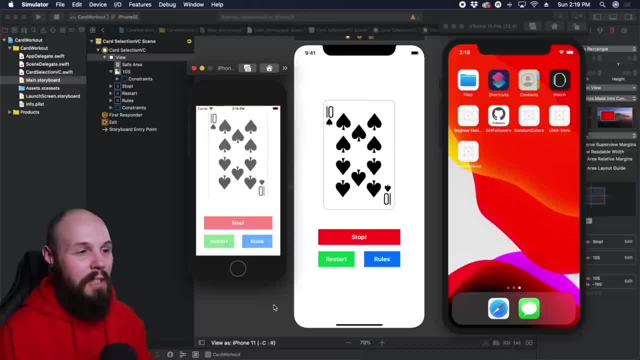 And we'll see. It should be fine, though It might be tight. It might be tight, It's pretty tight. So what we can do here is, instead of moving the card up 100 points, maybe we'll only move the card up like 80 points. 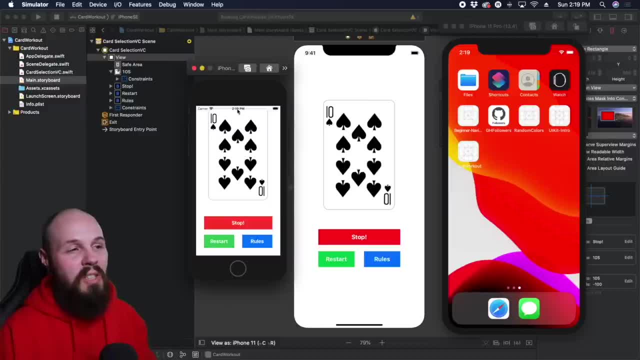 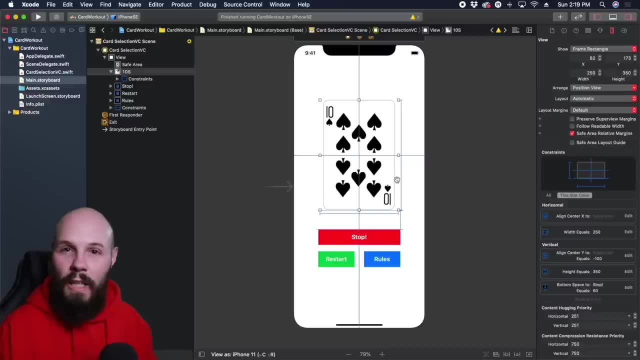 or 70 points from the center vertically Right, Because you can see it's just clipping the top a little too much. So let's make that quick adjustment Again. stop all the simulators Back here, And this is what I was talking about. 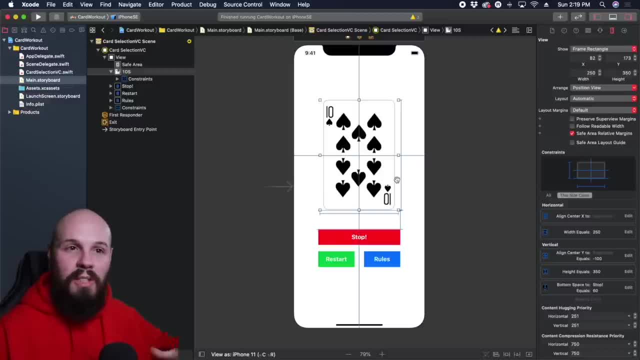 Remember how earlier I said, auto layout will do 90% of the work, but sometimes you may have to make small tweaks per screen size. This one we can actually make a tweak and it'll work globally. Again, right, If we change this align center Y here. 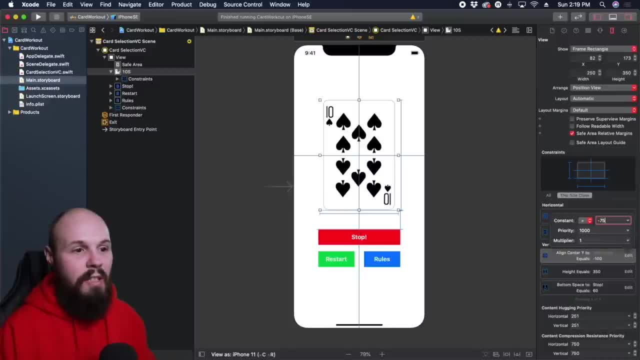 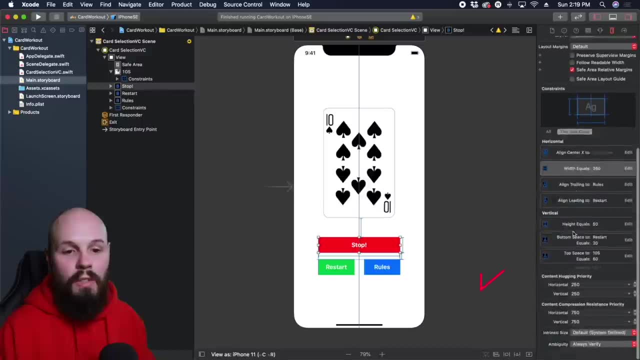 instead of minus 100, let's go minus 75. Just to bring that down a little bit. And then what we can also do is the top of the red button. we have a lot of space in between, So if I scroll down here on the red button, 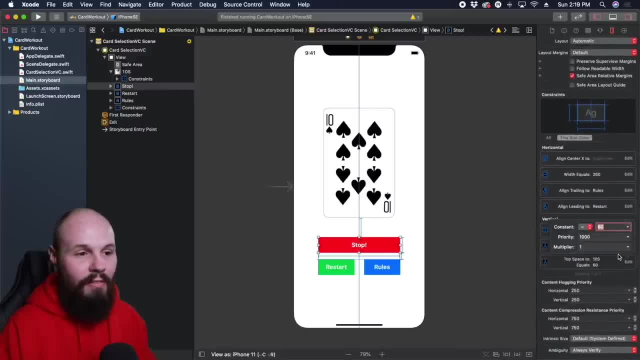 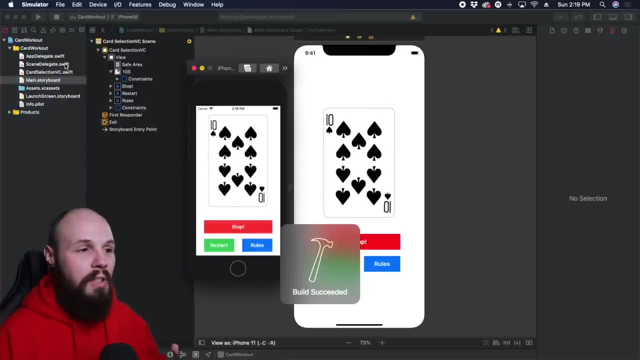 you can see, top space equals 60. Let's actually make that 50. There's a lot of extra space there. So now by doing this, by running it on the iPhone SE, that should compact that a little bit and be good to go. 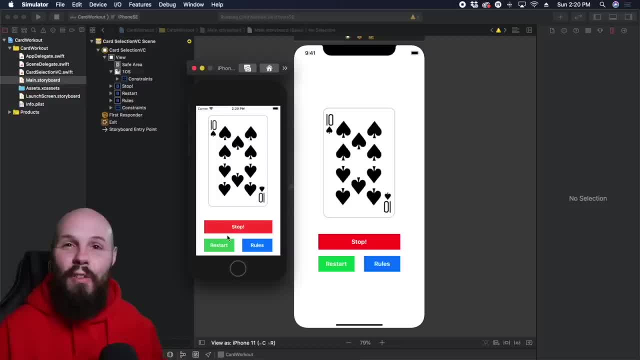 Yep, there you go. It's tight, but don't get me wrong. If you're designing for the big phones, you're going to accept a tight squeeze on the iPhone 5,, just as long as it's usable and doesn't look horrible. 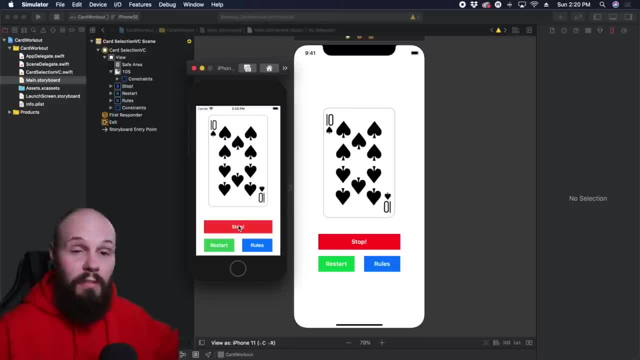 But that was a case where I could make a change and it was going to be fine on all screens. But you can start to see how I may want to make a small tweak just for the iPhone 5 and not have it affect my other sizes. 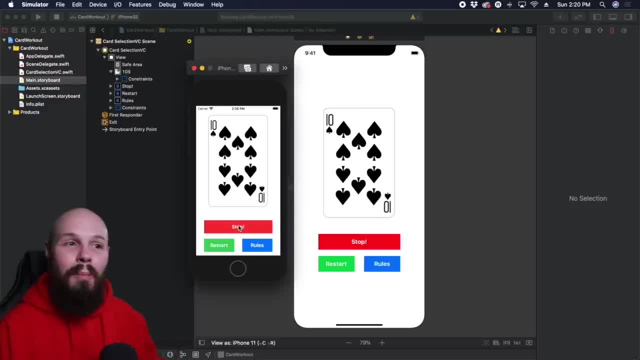 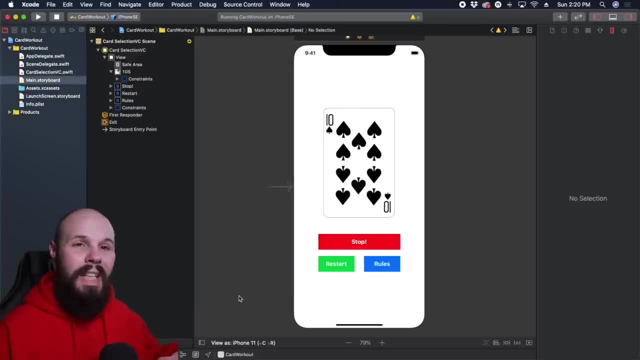 So, again, that's where auto layout does 90% of the work, but you have to get in there to really dial in and fine tune if you want your layouts to look perfect on all screens. That wraps up this video on getting the basic layouts. 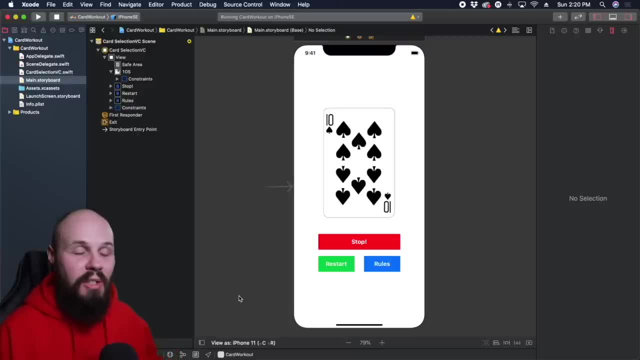 In the next video we're going to start hooking up our outlets and actions from our items on the screen to the code. As usual, here we are right where we left off, But, like I said, in this video we're going to start connecting our storyboard. 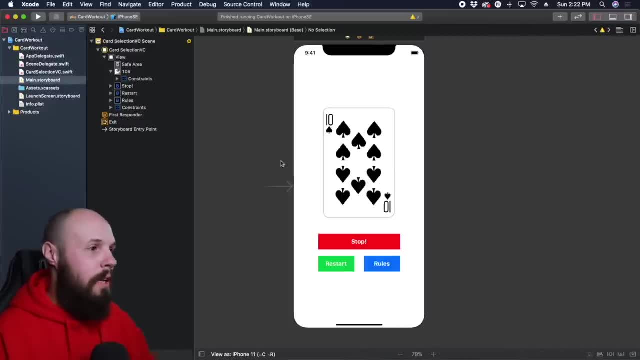 objects to our code. So here I'm going to minimize the right panel. Let's start making these a little smaller again. I'm going to open up our card selection VC and then I'm going to hold Option and click on the main storyboard. 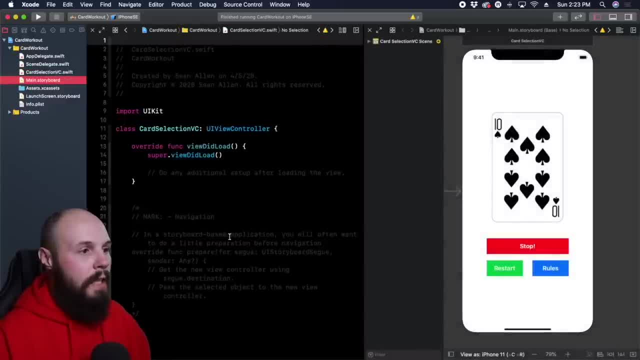 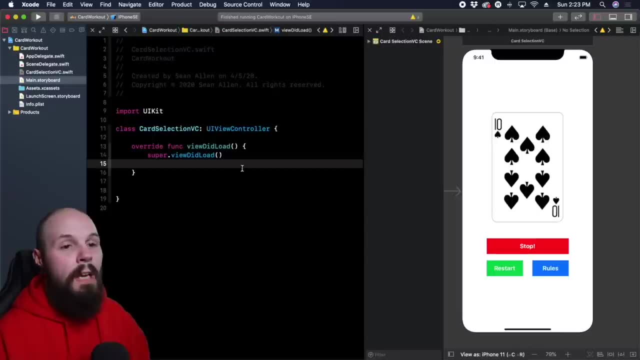 to again pull up the storyboard over here on the left And here in our card selection VC. I'm going to get rid of these comments, just to clean that up. Get rid of them, Okay. so the first thing we're going to do, 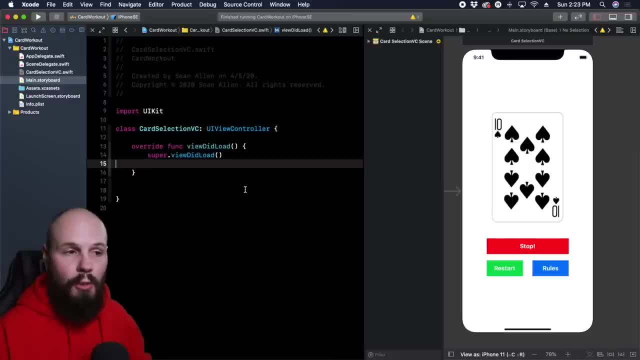 is create an outlet from our card image view. There's a difference between outlets and actions. What we did in the last video when we set up our temporary button, was just a quick IB action. Let me actually set these up and we'll start talking about the differences between the two. 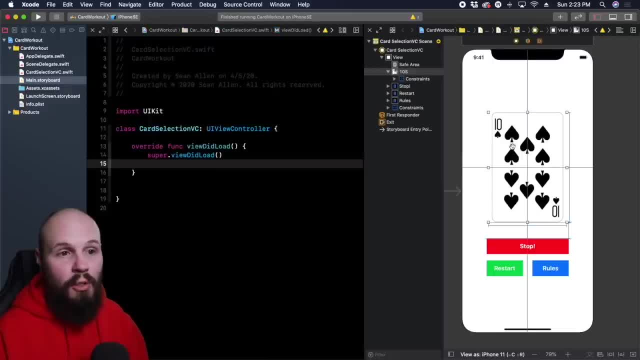 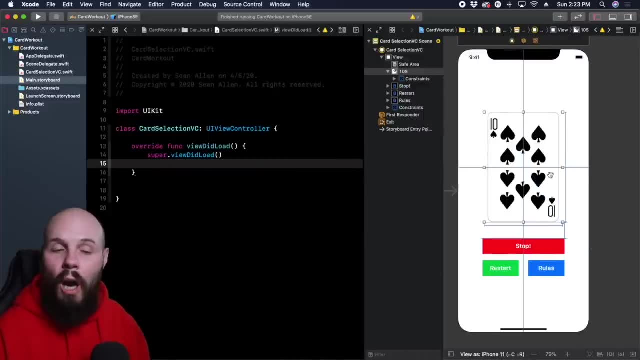 So again, to create these outlets, click on the card image view Control-Drag and you can see Insert Outlet or Collection And real quick, let me get rid of that. You can do it from the object on the screen, but if you have a real cluttered and busy screen, 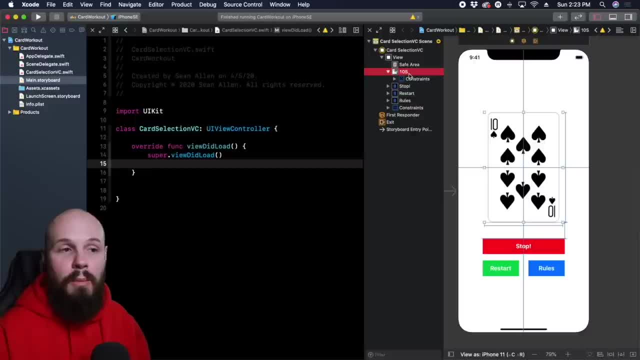 you can also do it from your view hierarchy. So here you can see I have the Ten of Spades image view selected. I can Control-Drag from the view hierarchy and also create my card And my outlet from here. We want to create it above view to load. 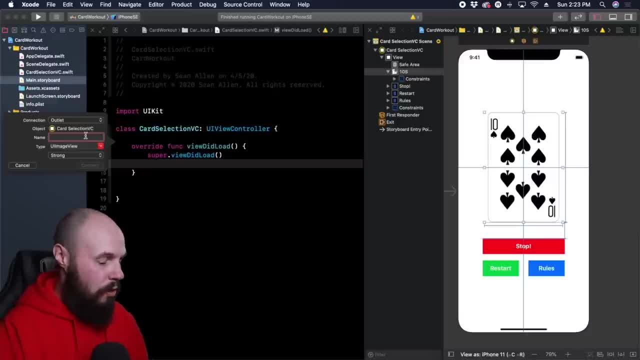 So you can see this is going to be an outlet, And again in a second I'll explain the difference. So the name is going to be Card Image View And it is a view by image view. Now you want to make your outlets strong. 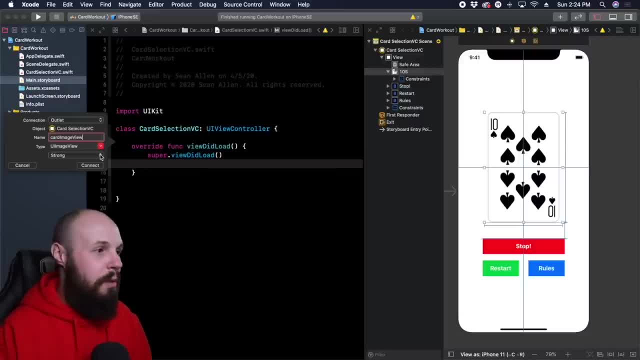 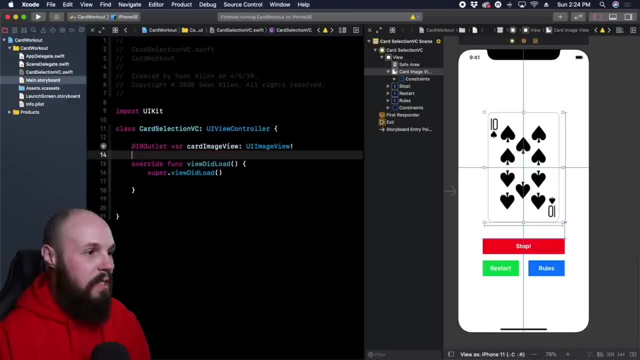 Xcode by default makes them weak. Let's flip them to strong. An Xcode engineer has said: no, they should all be strong. I followed him on Twitter and all that stuff. There was a debate, So change that to strong, Hit Connect. 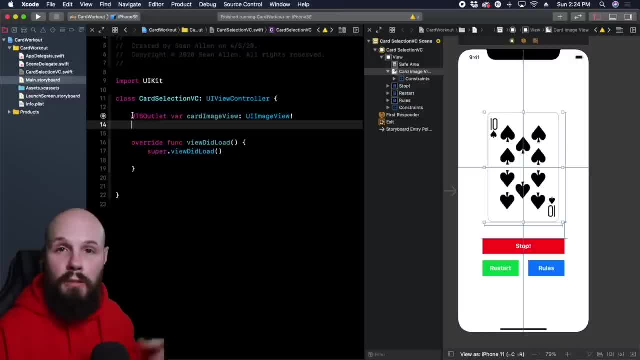 And again, make some space in between your view to load here So you can see where your view controller should go, And you're going to start to see that Your variables should be at the top. Then your view to load view will appear. 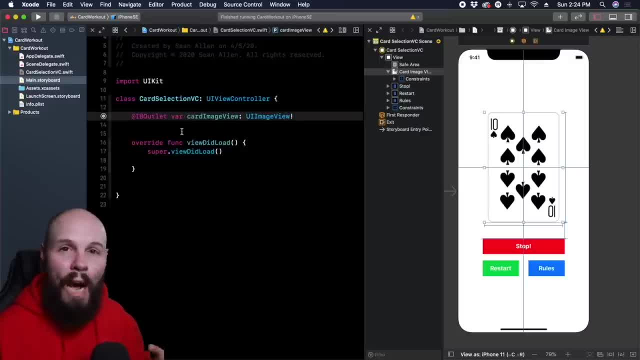 And then your functions. So you're going to see me put my variables and outlets at the top. So what an outlet does, Let's back up, Because you're already familiar a little bit with an action. Remember what an action does was. 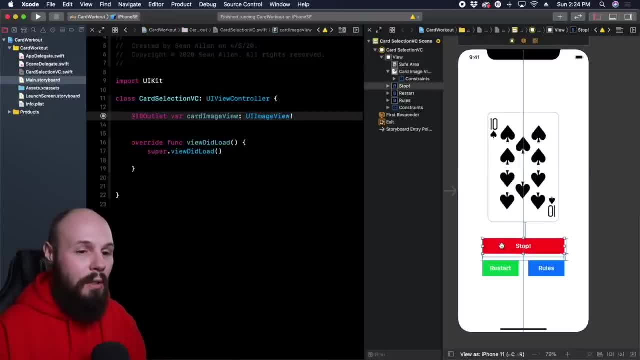 hey, when I tap the button, Actually you know what Easier to explain if we actually have one. So let's control-drag from the stop button here And we're going to create an action That is a UI button. 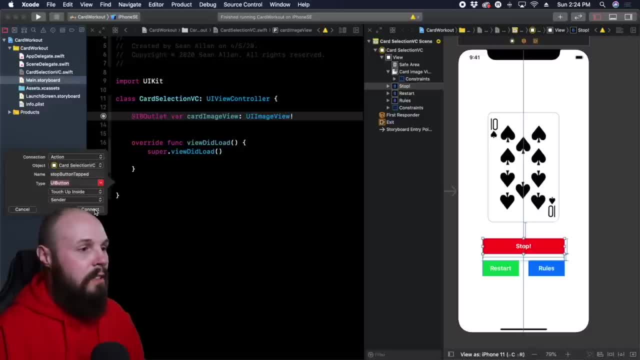 Again, touch up inside and sender. Those are the defaults. That's fine, Hit Connect. So here now we have an IB action. So now I can explain the difference. So the action, like you see here, is what happens when the actual button is tapped. 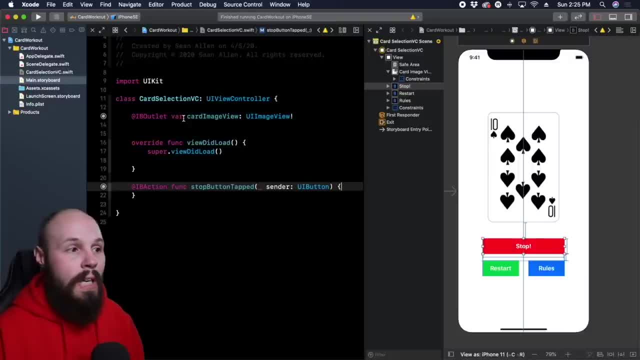 The outlet is what gives you access to this object in code. Right now I have access to card image view, This UI image view, And the reason you need access to that object is so you can make changes, So I can do image equals. 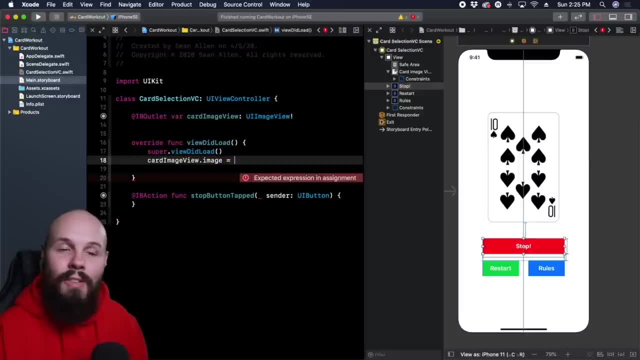 and now I can put in an image there. Now I can make changes via code. I don't have to make the changes on the storyboard Which you know you're going to see here, because we're going to change the card image view on a timer. 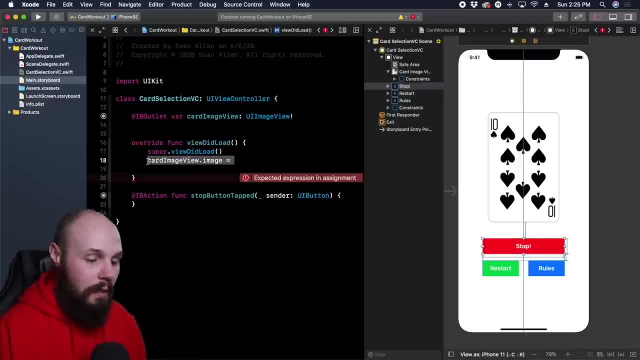 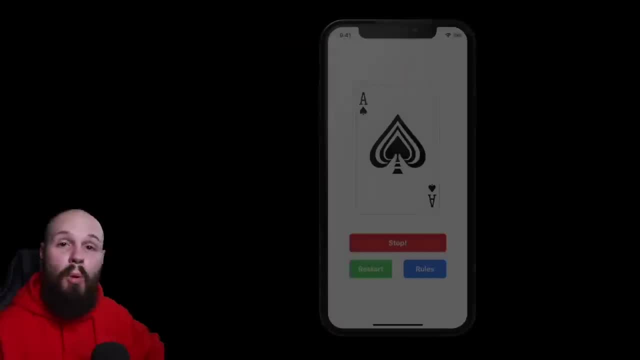 So that's how it like: shuffles through the cards. So an outlet, remember, is what gives you access to that object in your code, Not just on storyboard. And let's walk through an example of that right, Pulling up the design, you see that our buttons. 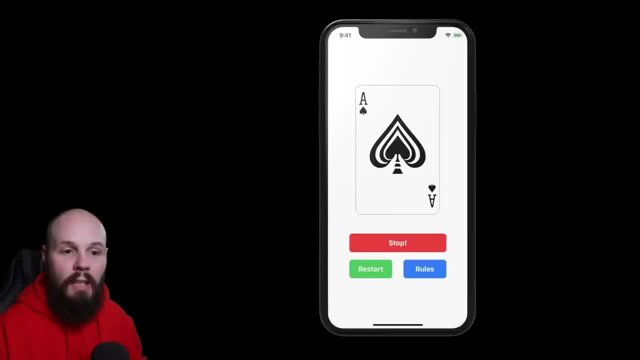 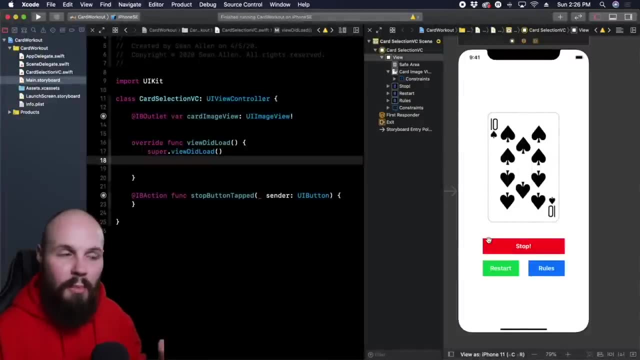 our stop button, our restart button, like you see on our storyboard here. You know they have rounded corners. There's a corner radius here. That's a styling choice. Well, I can't do corner radius in storyboard. That's something you have to do in code. 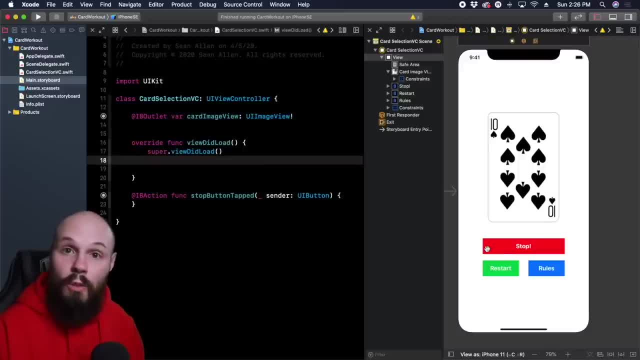 So in order for me to have access to these buttons in code so I can make that edit, I have to make outlets to them. So here we go, From the stop button. we're going to call this stop button. Pretty good naming. 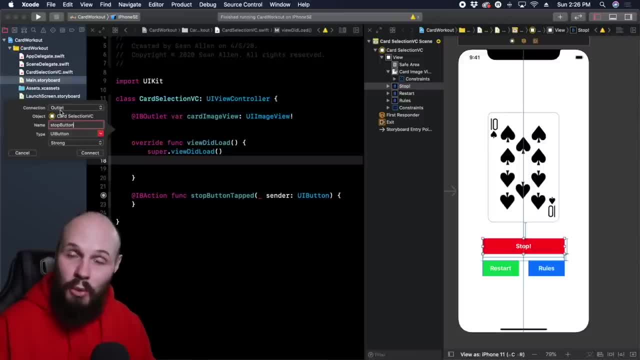 And again, make sure it's an outlet, not an action. So again, action is when you actually want to do something, when that button is tapped, And outlet is to get access to it so you can change the properties of it. So is UI button Again, strong. 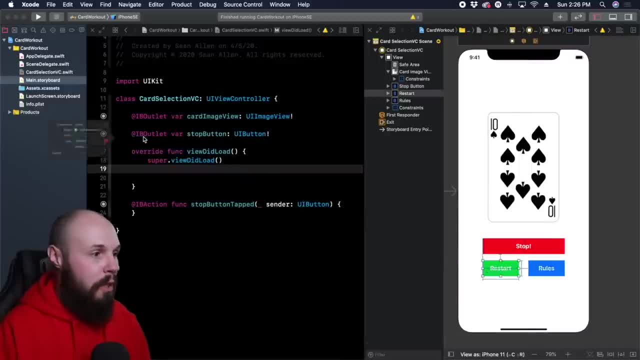 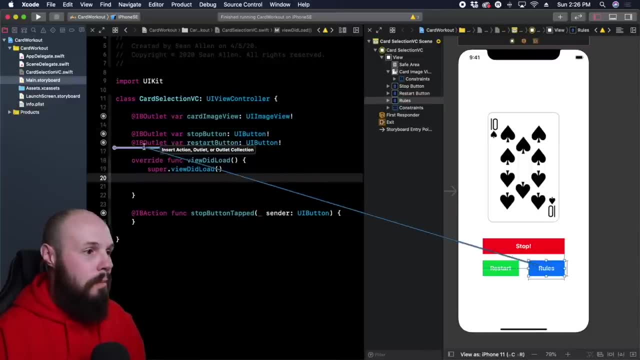 And again, we're going to create an outlet from the restart button. So restart button, It's a UI button, Strong Connect, And same thing for rules, Rules button. And now you see we have outlets for stop button, restart button, rules button. 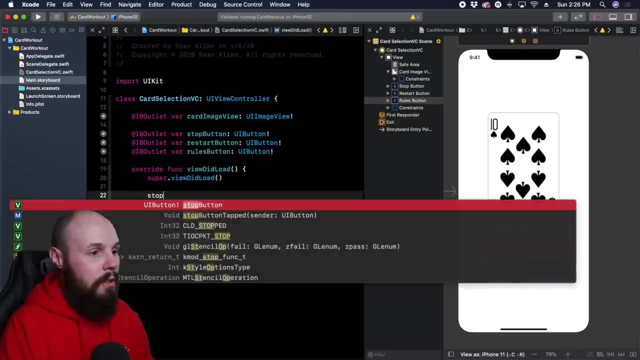 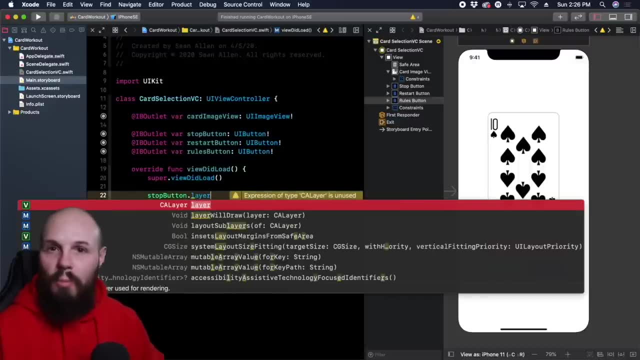 And let's give it that corner radius So we can do stop button, dot layer. This is a CA layer. When you're doing corner radiuses you have to go down to the layer of the view. Probably too much for the super beginner corner. 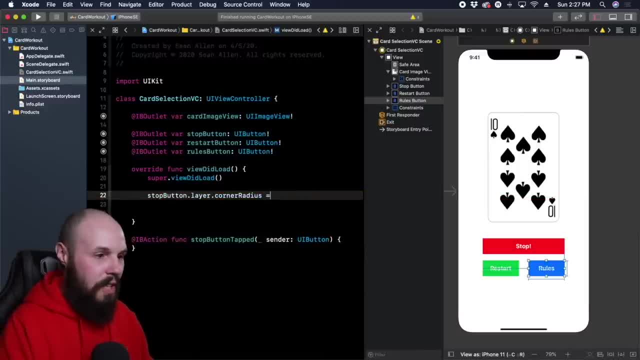 Of course, just know, the layer dot corner radius equals 8. And we're going to do this for the rest of our buttons. So copy and paste, And then I can double click there and do restart button Enter. Double click on the stop button. 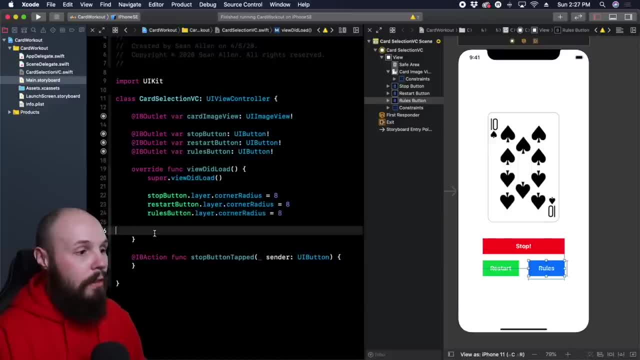 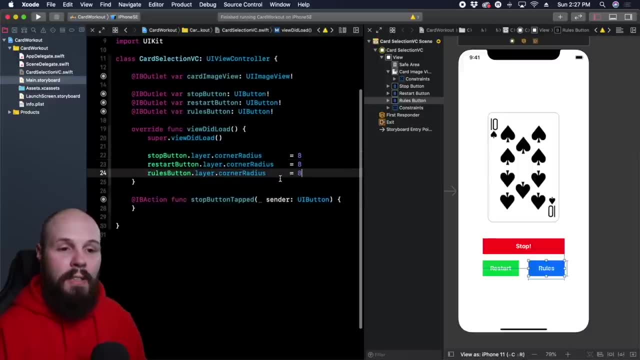 And then call it rules button, Enter. So now in ViewDidLoad you're going to see we're setting the corner radius of our buttons to 8.. So before we had sharp buttons, now we're going to have these rounded corner buttons. Let's get off the iPhone SE. 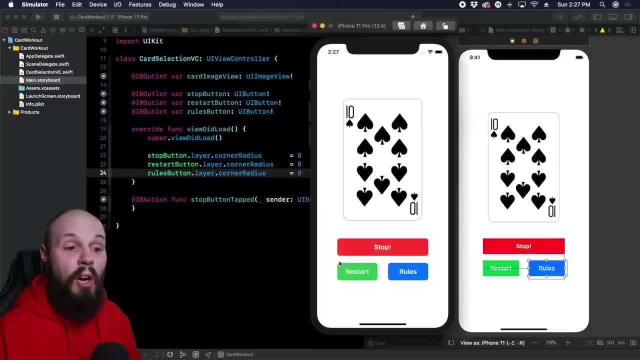 I don't even like looking at that thing, So run it Now. here you can see on our app our buttons are nice and rounded, whereas before they were sharp corners. You can still see those sharp corners on the storyboard. So again, when you want to make property, 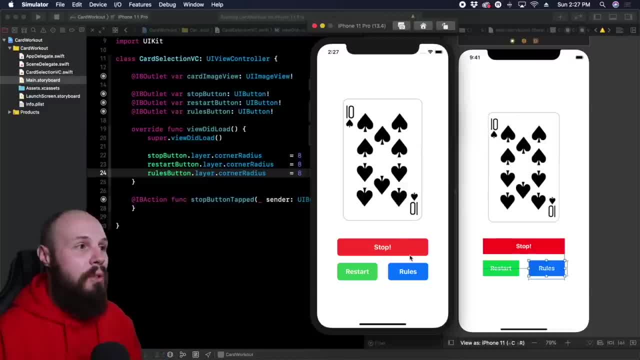 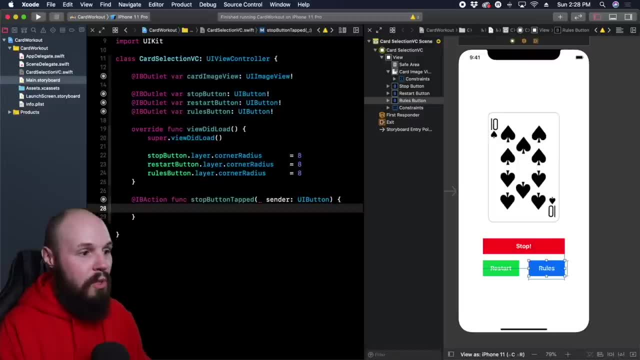 changes to the buttons. you need an outlet to have access to it in its code And it's not just the initial styling, Like, let's say, you know when the stop button is tapped, we want to change its name, So we want to do. 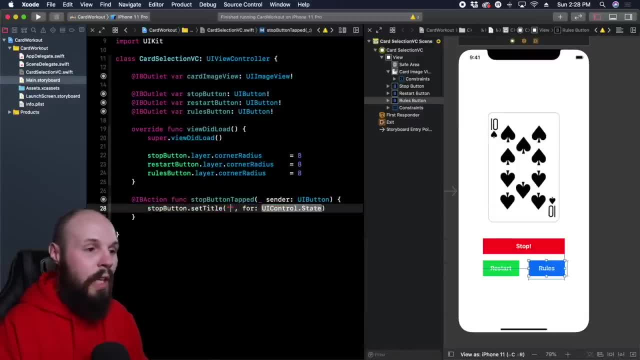 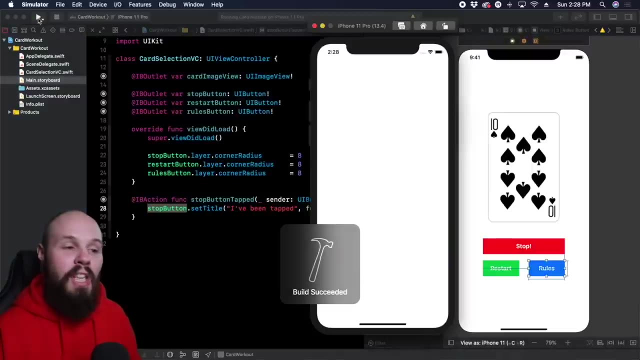 stop button: dot set title And we want the new title to be: I've been tapped for dot normal, So now I have to have this outlet to have access to this stop button. So now, when you see, when I tap the stop button, I'm going to change the title. 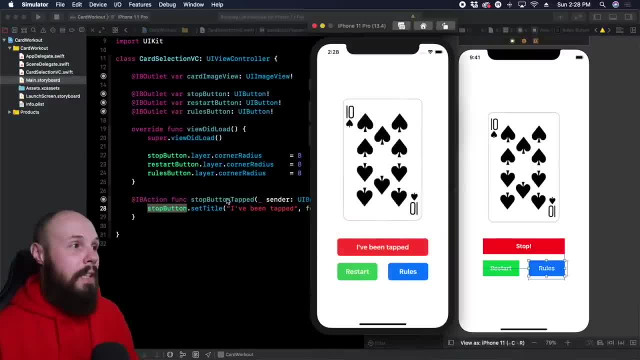 of it. So see, stop, I tap it, I've been tapped, There you go, So again. that's why you need outlets. I know I'm like really reiterating this, but I really want to drive the point home, for 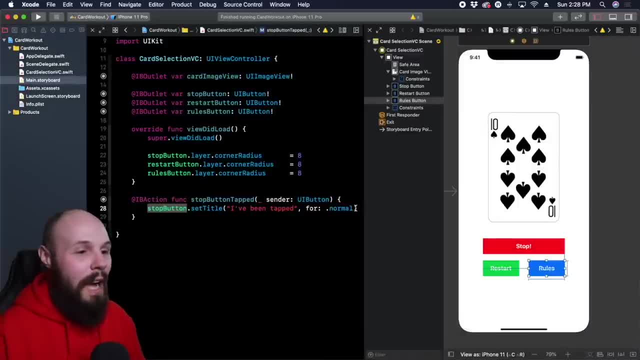 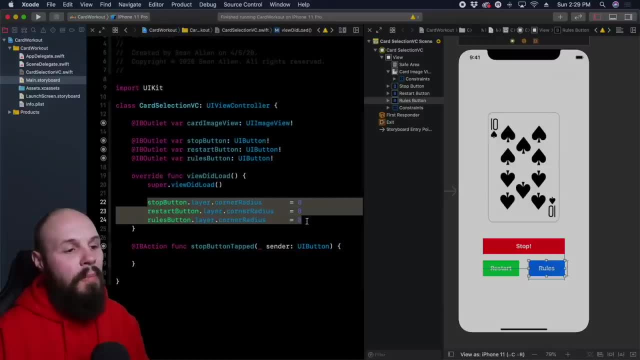 the thousandth time. Okay, So that is the outlets explained. We're not going to do that there. Now there's a couple things about this code that might stand out right. It's a little bit repetitive. There's a concept in programming called 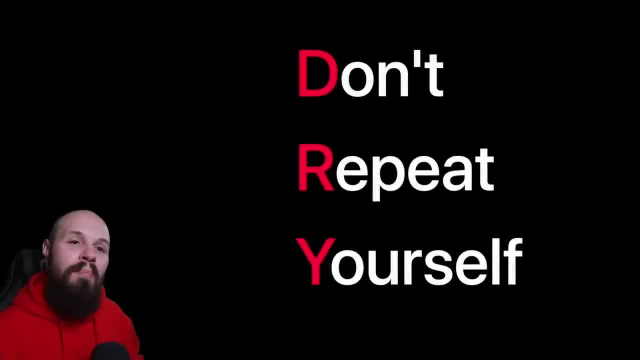 DRY like: don't repeat yourself. It is a rule of thumb, meaning it's not 100% absolute. You should never repeat yourself. There's certainly situations where having a little bit of repetitive code is better, but you know for the most part. 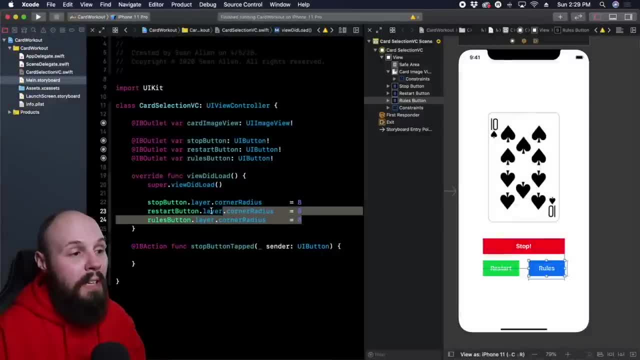 you should try not to repeat yourself, And this is an example of us repeating ourselves like doing the same thing over and over In the programmatic tutorial. we're actually going to create a subclass of this UI button. that is our custom class that is going to have all the styling in it. 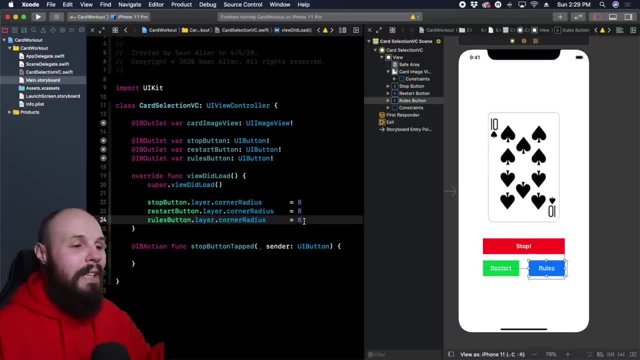 in the custom class, But that's going to be in the programmatic version. Here I'm going to show you a way to clean this up via storyboard. So, just like we had an outlet for these individual items, we can create what's called an outlet collection. 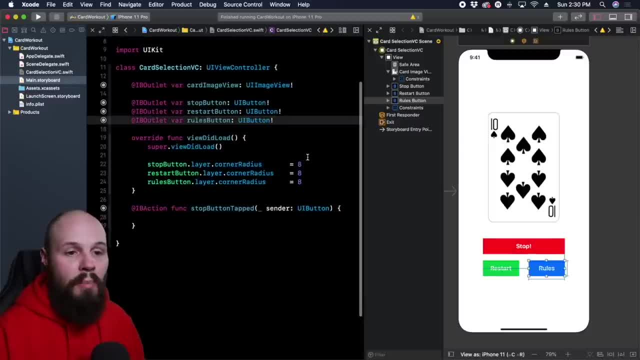 which is an array of outlets. So let's do that real quick. So from this button here, this stop button, control, drag again. we're going to create another outlet right underneath it and you can see insert, action, outlet or outlet collection. So let go of the mouse. 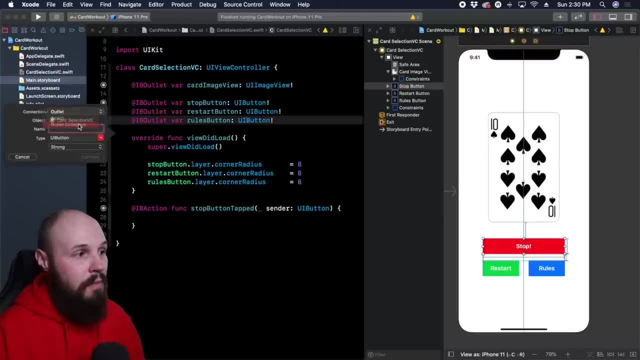 button first. So instead of outlet, we want it to be an outlet collection, right, And now we're going to name this. we're just going to name this buttons because it's an array. So pretend you're naming an array here, so you want it to be. 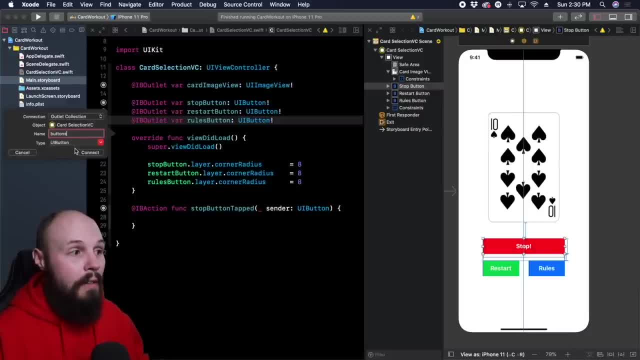 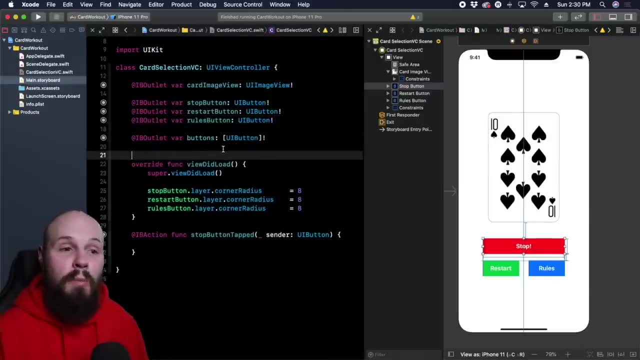 plural and you have to give it a type. So this is going to be an array of UI buttons. So you hit connect an array of outlets of UI buttons So you can see right here. So now we need to put certain buttons in there. And the cool thing- 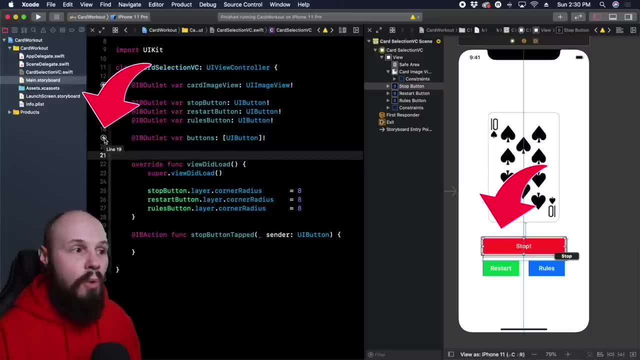 is if you hover over the little dot next to the outlet, you can see on the storyboard which ones are in there, Like, look, I'm going to hover it and stop hovering it. You can see. So we know we have the red button in there. So from the outlet, 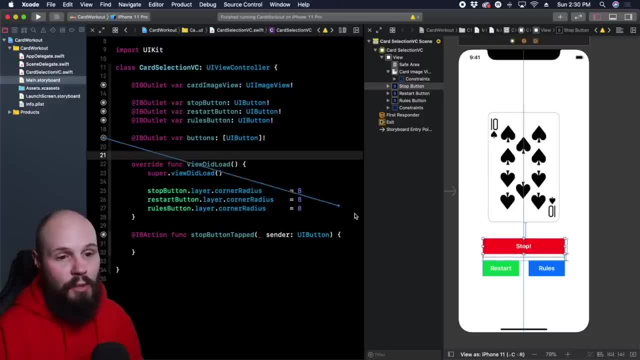 circle in the code you can drag to your other buttons. So watch, I'm going to drag this to the restart button. Now, the restart button is in my array of UI buttons And the way you can see what's in there, hover over. 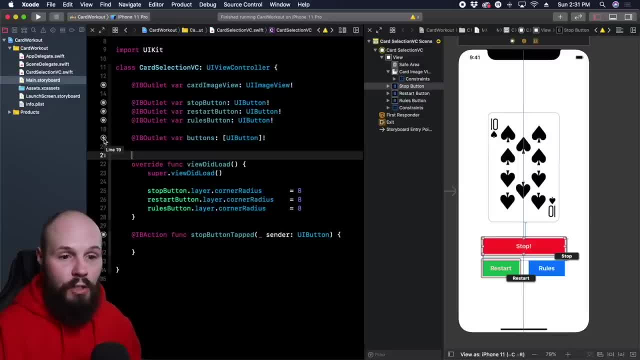 that, and now you can see. the restart button and the stop button are in there. Now let's drag and include the rules button. Bam, Now this IBL collection has all three of these buttons in it, So now what I can do instead of. 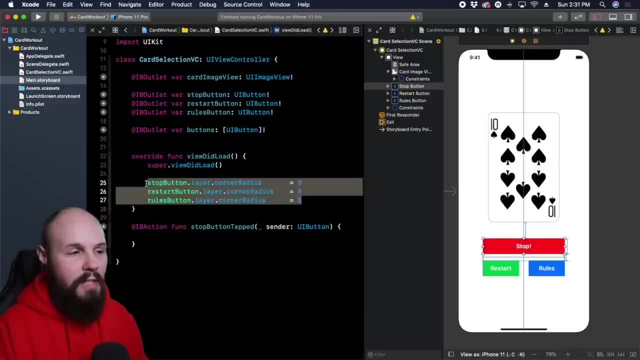 writing this code out three times and you're going to see this isn't going to save many lines of code, but you can see how if we added more buttons to this it could get kind of ridiculous. But now I can use a for loop to iterate. 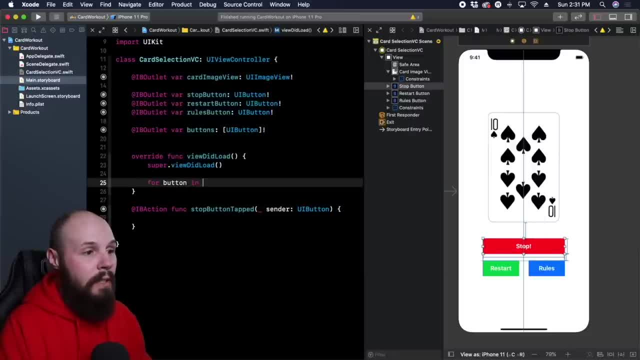 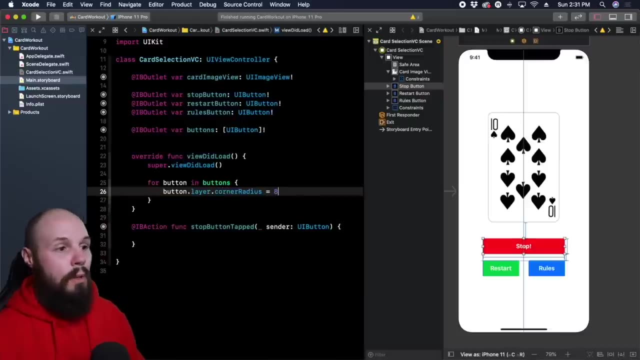 over that array of buttons. I can do for button in buttons, Again this buttons. here is this IBL that we created, which, as you can see, is an array of UI buttons, And now I can do button dot layer, dot corner. radius equals eight. So now, 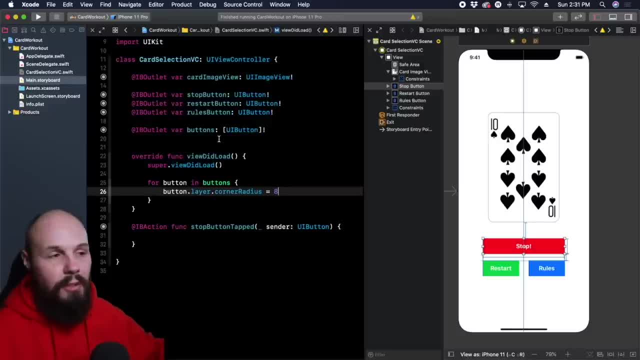 I can add, you know, twenty more buttons into that array, you know, if I wanted to. And this line of code doesn't have to change, because I'm iterating over every single button in that array and setting the corner radius to eight. So let's test this real quick. 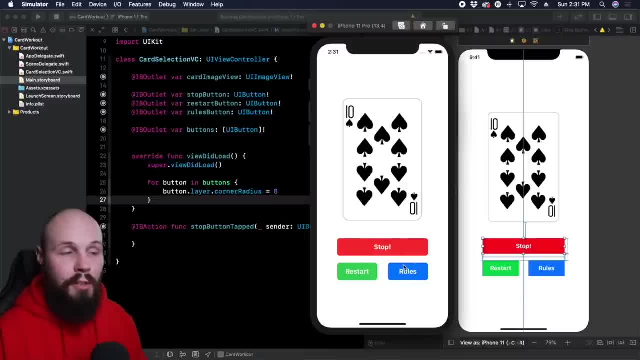 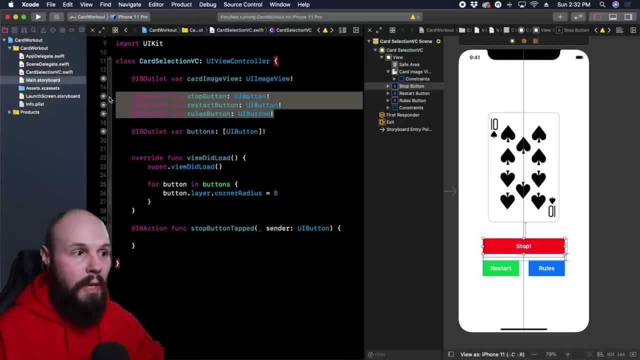 And here you go. The code works just the same. Our buttons are rounded corners. Now, something else we can clean up is we can get rid of these outlets here, for our specific instance, Right. Just because you put them in array doesn't mean. 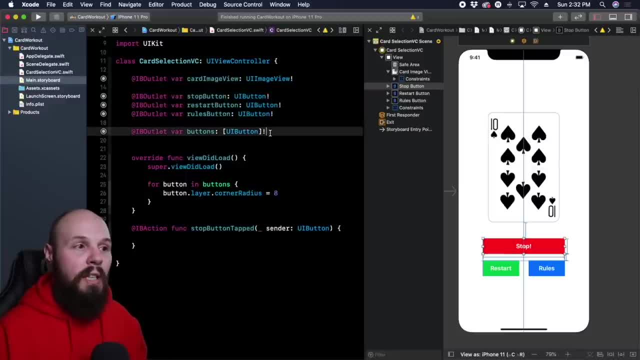 you can always get rid of them, But in our case, we're not customizing our buttons anymore. I don't need access to these. You'll see as we write out the rest of our code. we don't use them, So what I can do is: 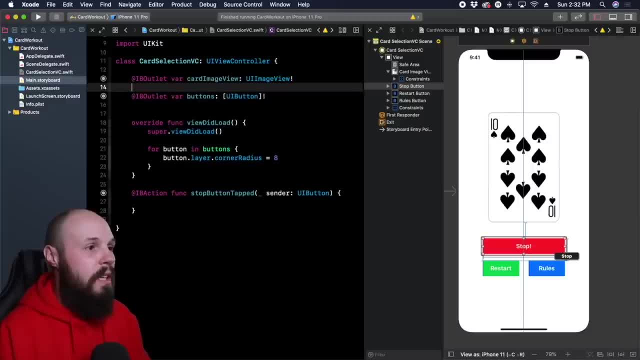 delete them. So we'll delete all those. clean up the code a little bit Now. we just have those outlets. Hopefully, alarm bells are going off in your head right now. I hope, based on what we did last video, right, I just. 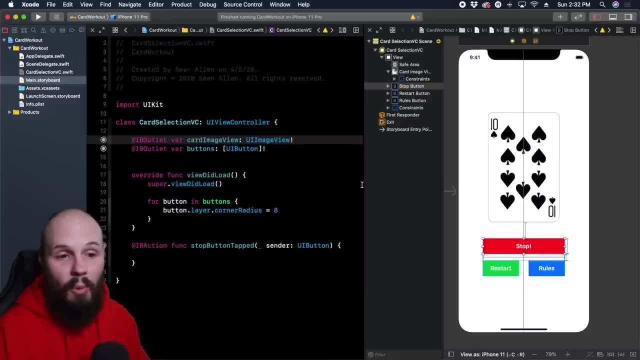 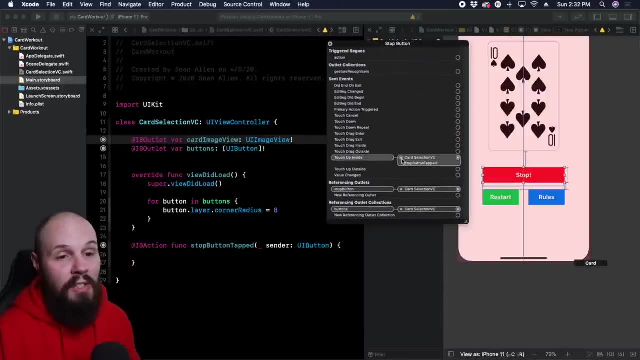 deleted those outlets. However, they're not deleted from the storyboard. So, right, watch what happens when I right click one of these buttons. now You can see our list of outlets here You can see. okay, so I have the action on the stop button, which is down here. 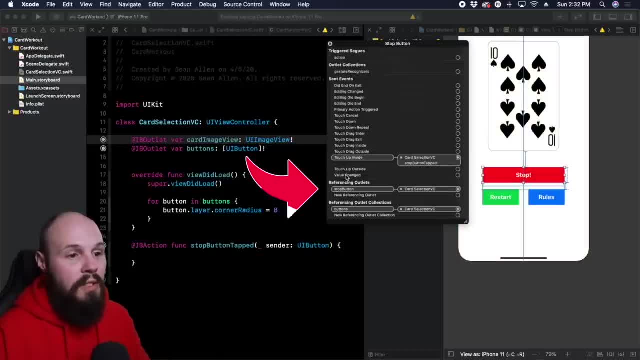 That's fine, We're allowed to have that. We want that Referencing outlet. You can see I have a stop button outlet. I have to delete this one because that's what we just deleted in code And you can see it's in an outlet collection. 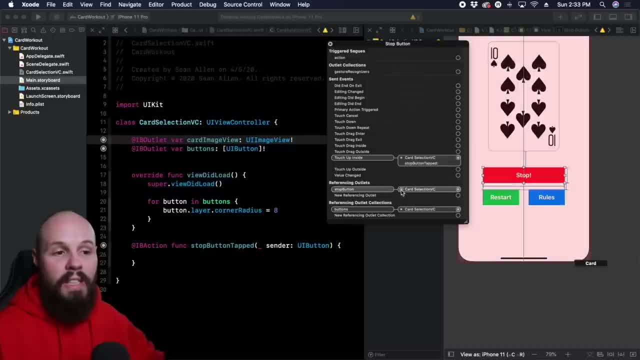 buttons. We still want to keep that, We want to keep it in our collection, but we want to delete the individual one that we had. So that's why, remember I said in that previous video: there are certain cases where you don't want to. 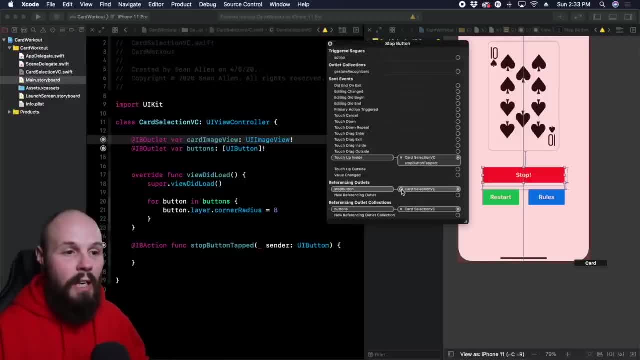 delete the whole button. You just want to delete a certain outlet that was attached to it. And again, I hope this sticks into memory. I want to pause right here. I've had so many beginners working with storyboard look for an error for hours that they couldn't 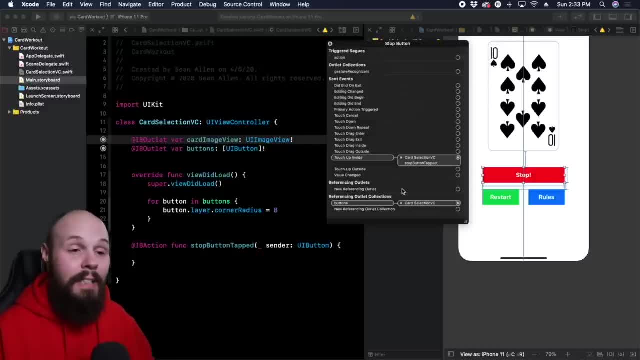 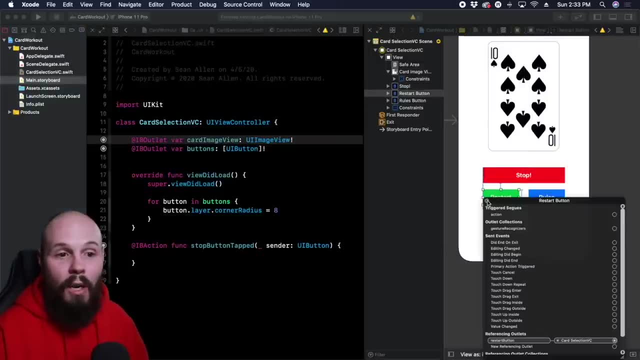 figure out and it's because they had some extra outlet attached that they didn't need. So always check to make sure you've cleaned up your outlets if you're having issues. So again, right click on the restart button. Here the referencing outlet We want to delete. 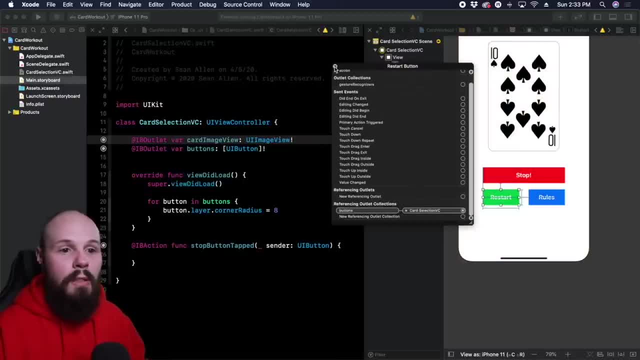 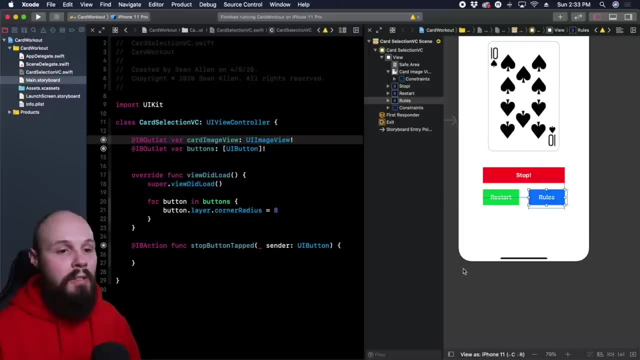 that Not the outlet collection, just the referencing outlet. Boom, Delete. And then on the rules here, right click that You can see here we want to delete the referencing outlet as well. So now we've cleaned up our outlets and we should. 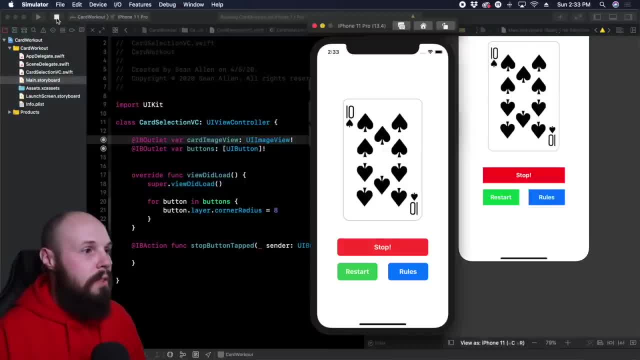 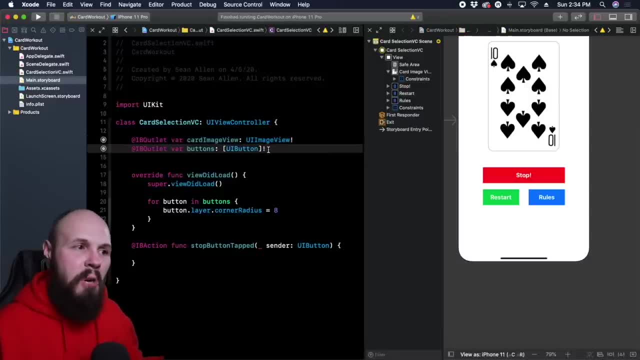 be good to go. Let's run it just to verify. And there we go, Still working. So a little bit of cleanup and an introduction to the concept of outlet collections, which even experienced programmers don't always know existed, Like I've shown this in a video before and I've had people say 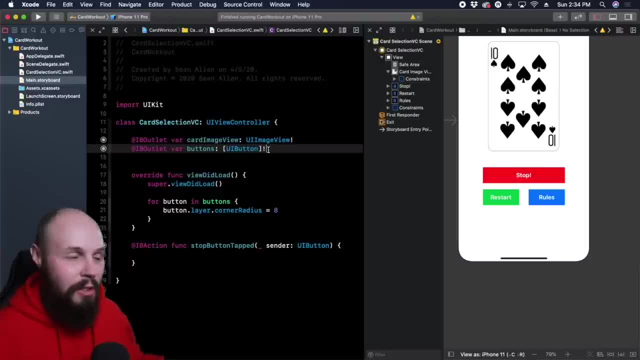 like I've been working for three years on this. I had no clue that existed, So hopefully you got something out of that one. Alright, so let's finish setting up our outlets here. Outlets and actions: We've set up all. 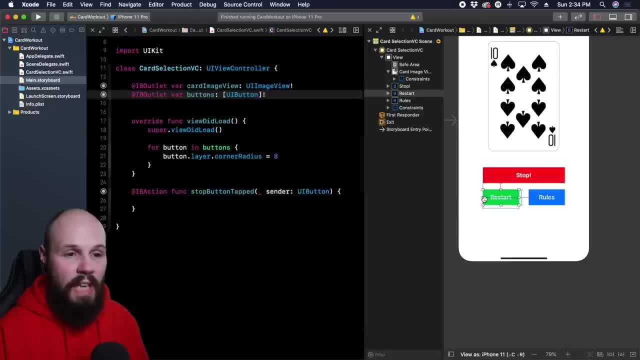 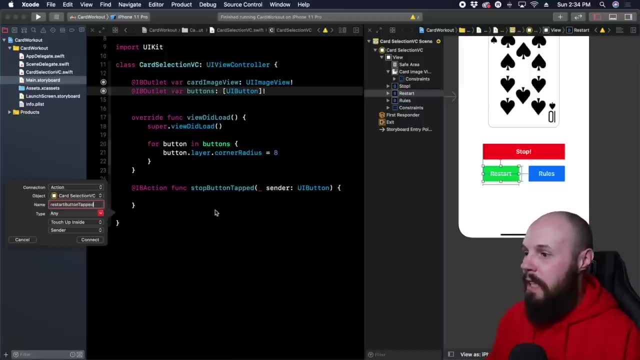 the outlets we needed, But we need more actions. right, We need restart button tapped. So let's control drag here, Let's create a restart button tapped And again, that is a type UI button. Touch up inside is fine, Connect. 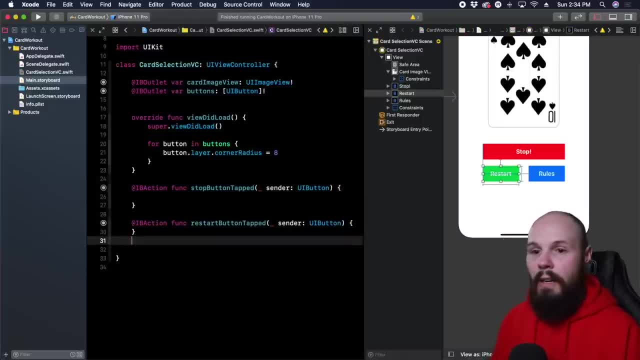 Make some space there. And now let's add our rules button tapped, And then this should finish up the outlets and actions that we need. So, rules button tapped Because, again, we want to take action whenever these buttons are tapped here. So again, IB actions for when you want something to be. 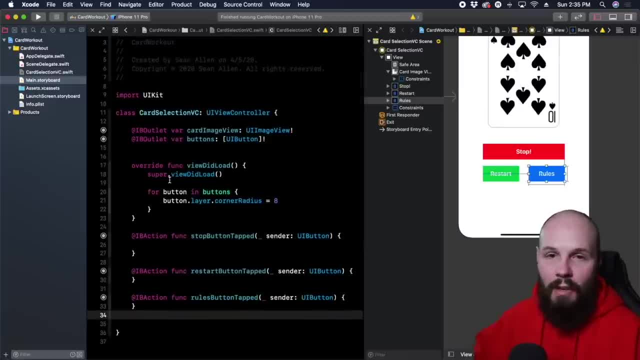 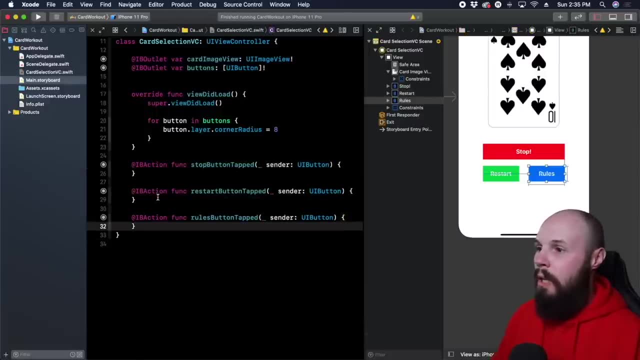 done IB outlet for when you want to access the properties of that object. So, as you can see here we're setting up our actions to write some code in in a later video, But our UI is set up almost almost, almost almost. 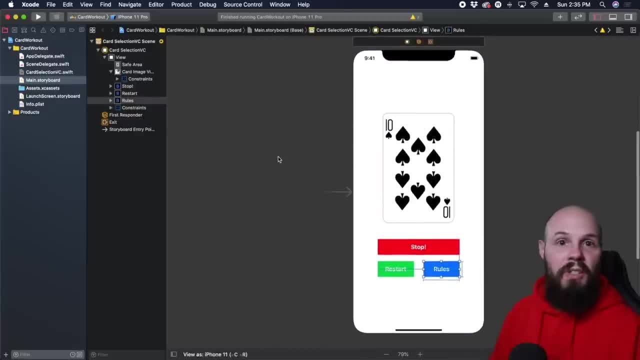 So let's close this one out and get back to our storyboard. We're missing a screen. Right When you tap the rules button, a new screen slides up and shows you the rules of our workout. So let's add that view controller. So I'm going to slide this over here to the left. 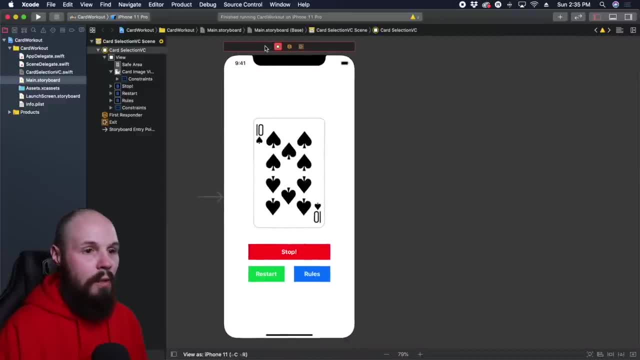 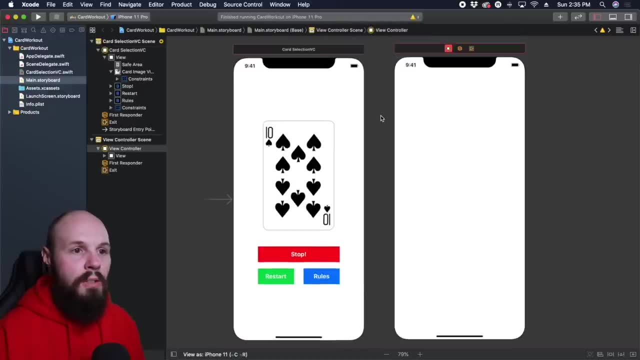 I'm just dragging around here on that bar And then again command shift L, Pull up a view controller. There we go, Drag it onto the screen. So there we go, And we want to present this modally, Remember modally. 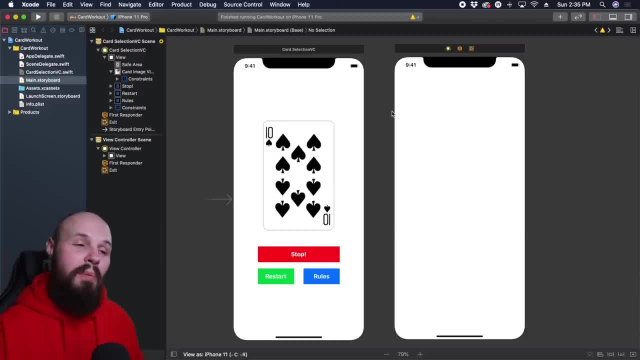 is when it slides up from the bottom. If we were in a navigation controller, it would slide in from the right, like we did in the previous app. So one thing with actions. If you remember, when we added that temporary button last time, We created an action from our button. 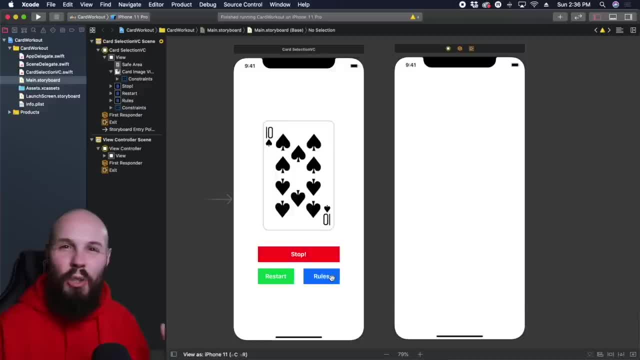 and then I typed in perform segue with identifier. I did that just to show you that If you're doing nothing but a transition from a button like, you don't have to pass any data or do anything else. you can just directly control drag. 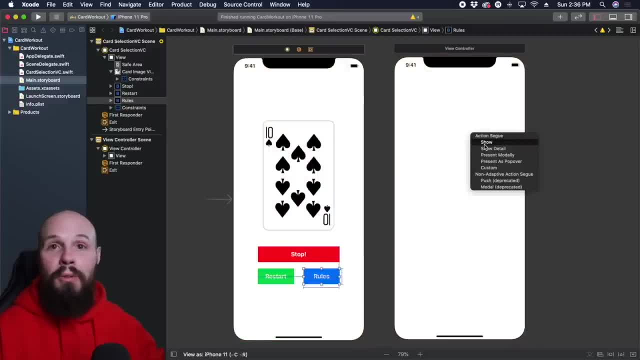 from the button to this view controller and it will create that segue to show it. Now watch what happens. So we want to present modally. That's what we want to do, But I want to illustrate something. If I do show. 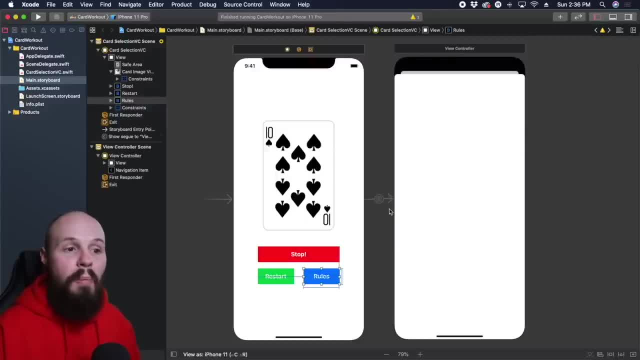 it's still going to create this segue here, but you'll notice, because I'm not in a navigation controller, we're not going to get the slide over effect. You only get that in navigation. Even though I picked show, it's going to slide up from the bottom. 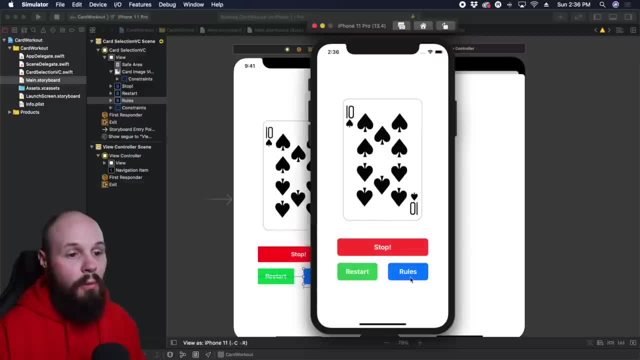 Watch. I'm going to run this here, So hit rules. You see it slid up from the bottom And then we get this nice iOS 13 card here, So we swipe it down. Rules, Swipe it down, Rules, Swipe it down. 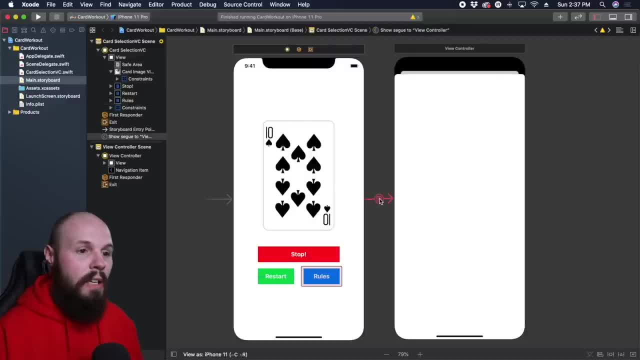 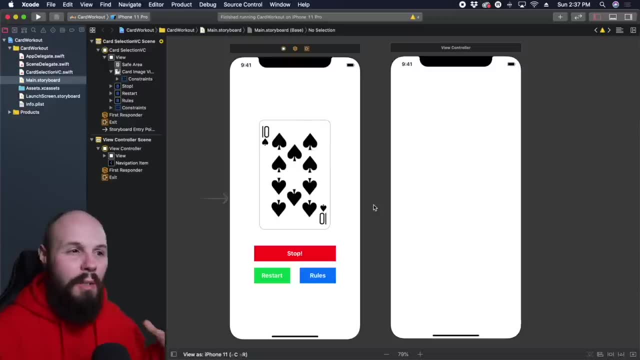 So let's close this. But I want to change this. I'm going to delete that segue And we want it to be present modally, just to avoid confusion, Because if an experienced developer comes in here, they see a show segue, they're going to be thinking: you know. 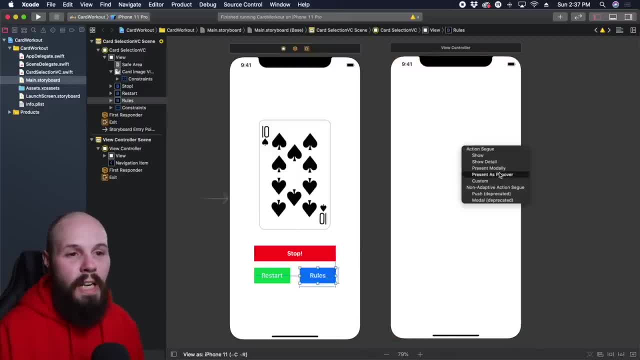 navigation controller. but why not? So let's name it the proper name here. present modally, And then again. before in the previous app we got the navigation bar at the top when we were in the nav bar. Now we're getting the card looking thing. 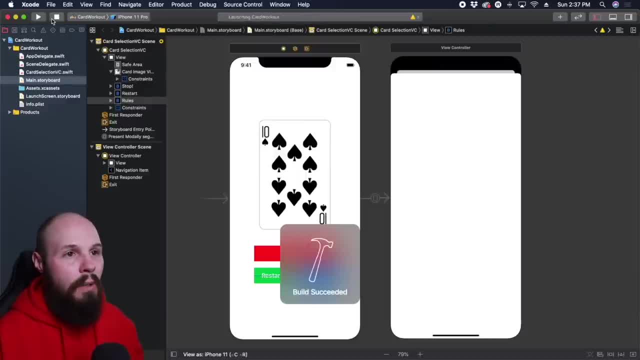 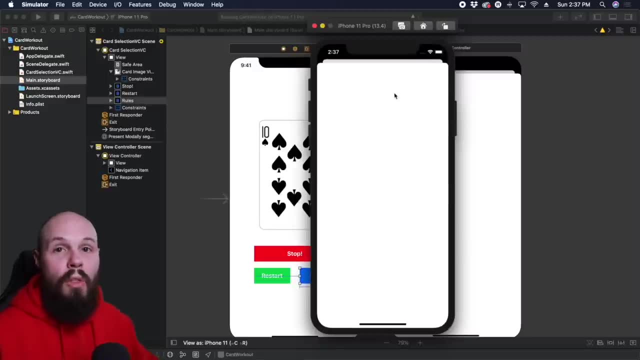 that's new in iOS 13.. So let's run this again, because I want to point something out, because we're sticking to iOS 13, because this changed in iOS 13.. So I tap rules and we get this card. I can dismiss this by sliding. 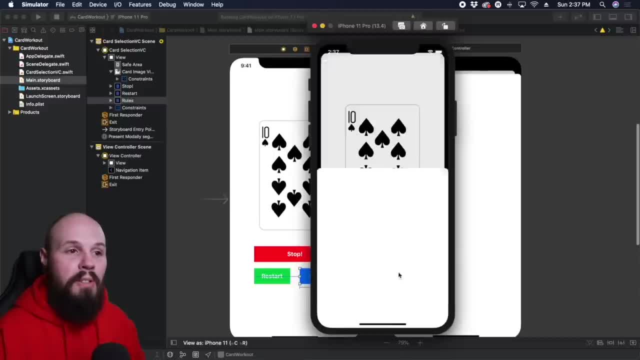 down. If you just drag and slide down, that's how you dismiss the modal pop-ups now in iOS 13.. If for some reason, you are doing this on iOS 12, like you can't upgrade to iOS 13 and Xcode 11,. 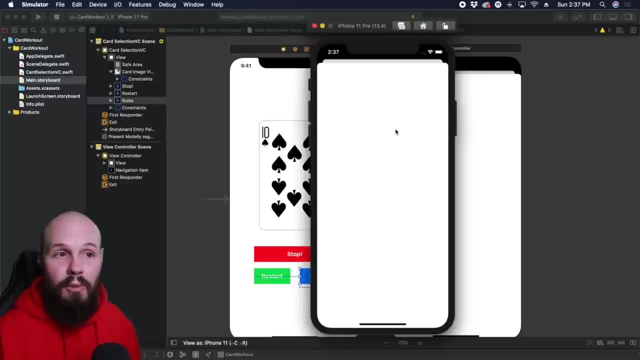 what's going to happen? you're going to tap rules and this is going to fill up the entire screen And you're not going to have this swipe down gesture to get rid of it. So if you are in that situation, you're going to have to add a. 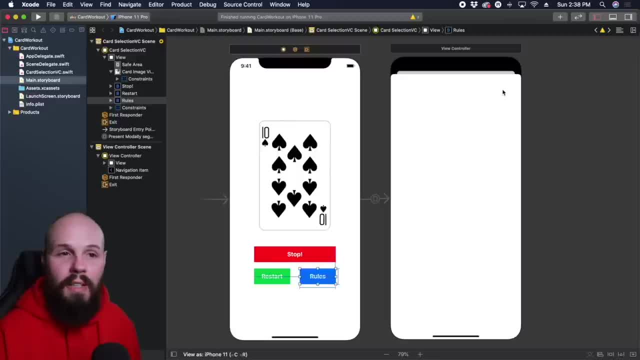 button to the screen to dismiss it. So you tap done or something like that, and then it dismisses. Maybe that's a little bit of extra homework And if you are in that situation, hopefully you can figure it out. If you can't figure it out, of course, leave a. 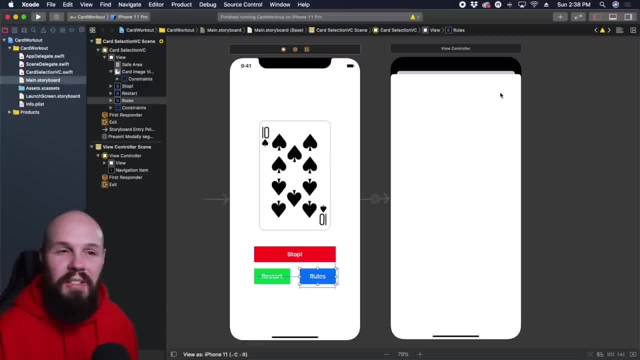 comment. hit up the Slack channel. Happy to help, But I think that's a fun little challenge to give those of you that aren't on iOS 13.. So, okay, we have our screen here. It's working. Now let's. 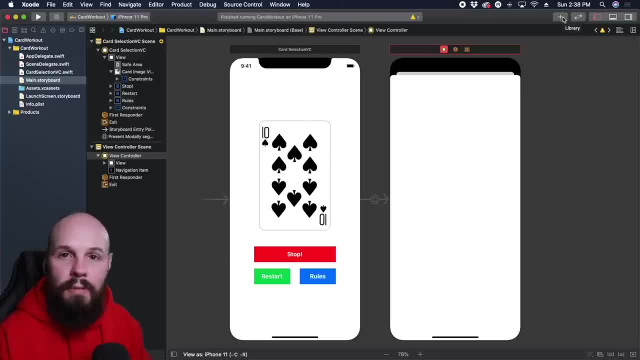 add our label that has all of our information, And actually it's three labels. So Command-Shift-L or hit this plus button, whatever you prefer, by now, Drag a label onto the screen here And now. we need to constrain this. First, we're going to open up our right pane. 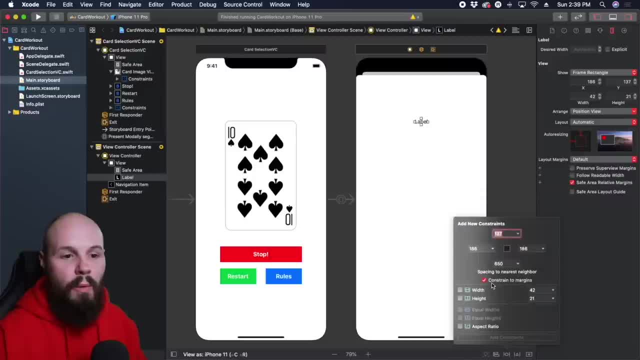 here And then down here, our little TIE fighter right. We want to not constrain to margins. Don't do that. We want to do 30 from the left, 30 from the right and let's call it 70 from. 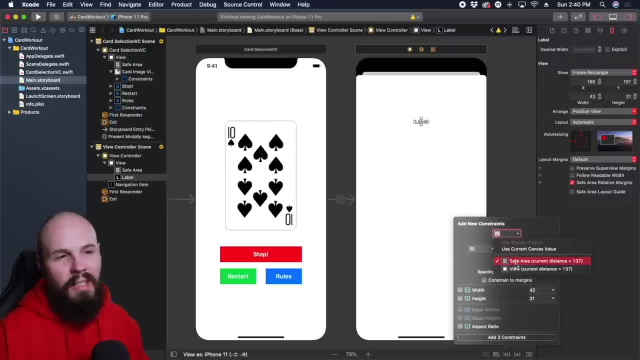 the top here And we will pin it to the safe area. Actually, the safe area doesn't matter because we're in our little modal screen slide down, but hey, it's the same distance: See view and safe area distance is the same. 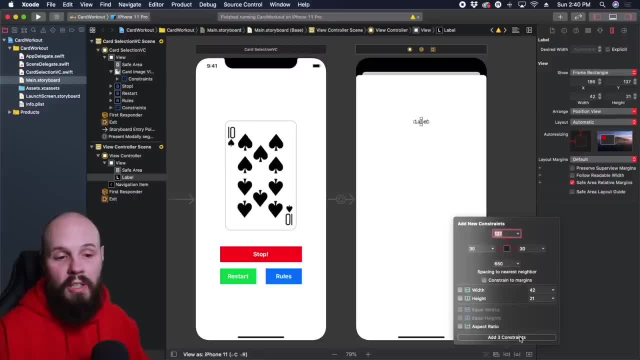 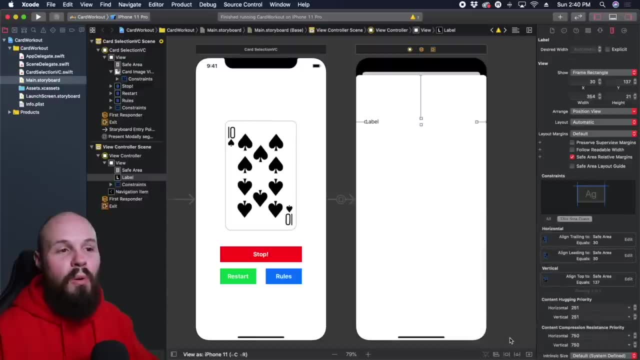 We'll keep it the safe area. So hit. add those three constraints. Now you could give it a height if you want, but again, labels have that intrinsic content size, So you don't necessarily need a height. Labels are one of the few that you don't need. 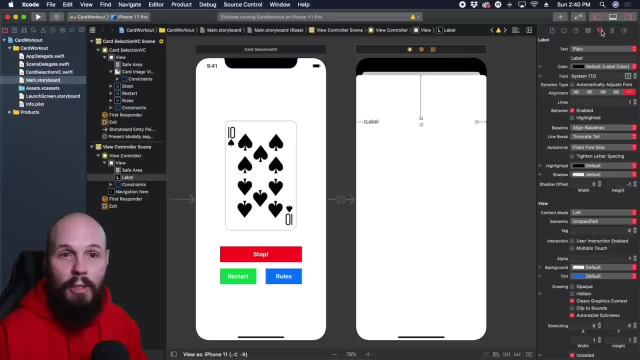 that. So, with our label clicked, let's type in or go to the attributes inspector. Instead of it being called label, let's call it rules, Hit, return. We want this to be centered, as you can see, in the alignment And our system size. 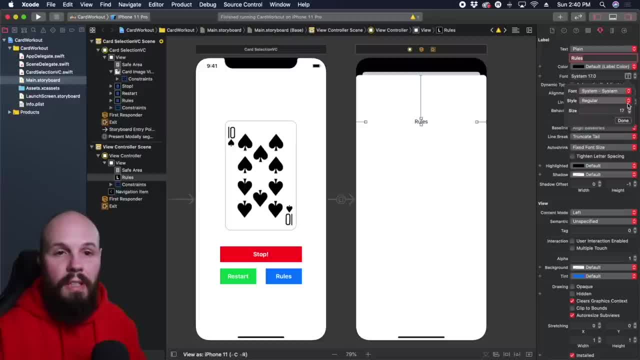 here. we're going to keep it. system font. That's fine, You can play around with the fonts if you like. Style: I'm going to go to bold And then font size: we're going to go to 40.. This is real big. 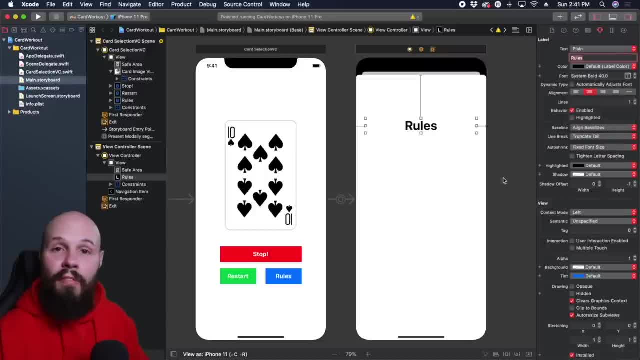 Rules right there And hit done. So that's our first label. Let's go ahead and do command shift L. Let's add our second label And let's constrain this again down to the TIE fighter. Same thing, 30 from the left. 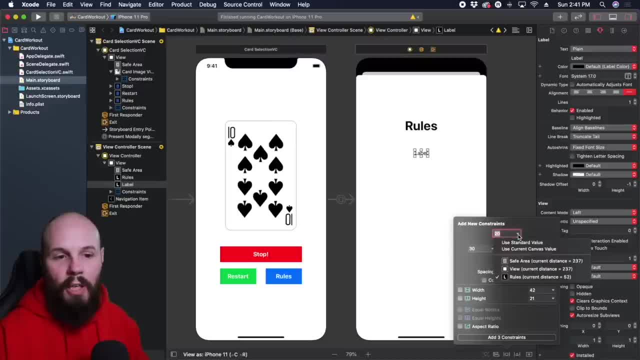 30 from the right And we're going to do 25 and hit the drop down, just to be sure Again from the rules label. So we're pinning this to the bottom of our rules label up here: Hit add three constraints. 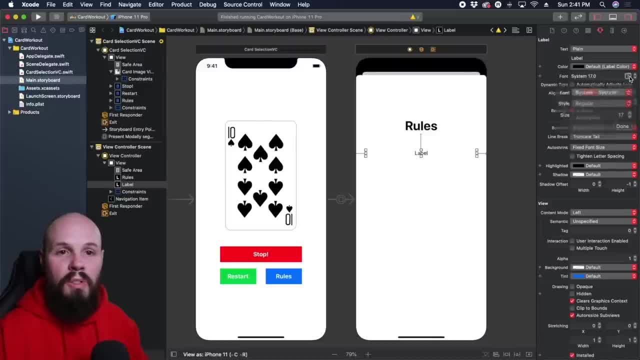 We also want this to be centered. We're going to go system semi-bold- Not fully bold, Semi-bold- And make it 18.. Hit done And now we need to type out our rules And we're going to type up here. 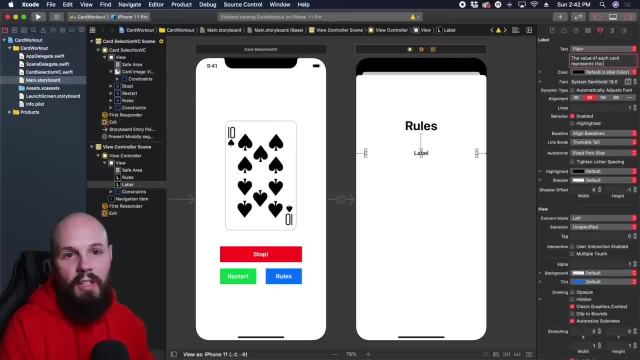 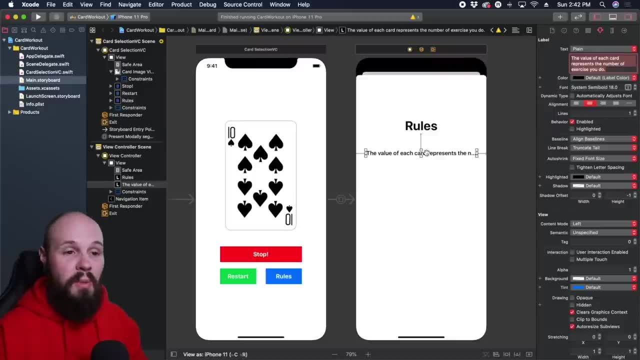 the value of each card represents the number of exercise you do: Period, Hit, return, Okay, well, that doesn't work, It doesn't fit right. We get those dot dot dots. Well, here you see line break where it says truncate tail. 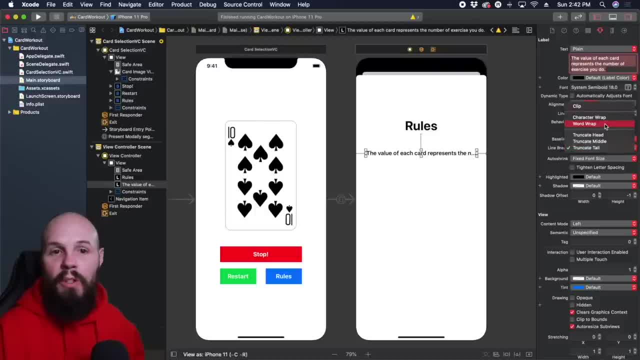 You can decide how you want your label to break up its lines. And we want to do word wrap And then here number of lines above it. We have set to one. That means it's only going to be one line. You can set the exact number of. 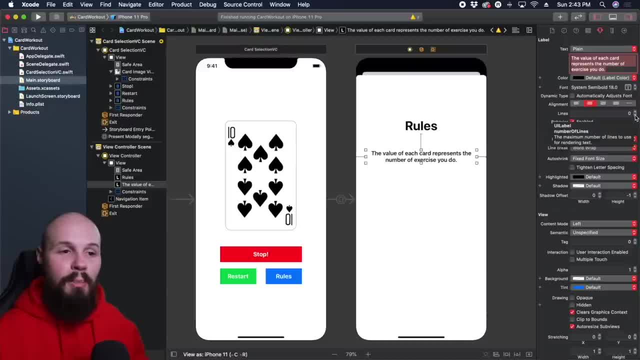 lines if you like, Or if you pick zero, it'll automatically adapt to the number of lines you have. Now we're missing a line, Like we need to know what the jack, queen and king are, So up here in our text here. 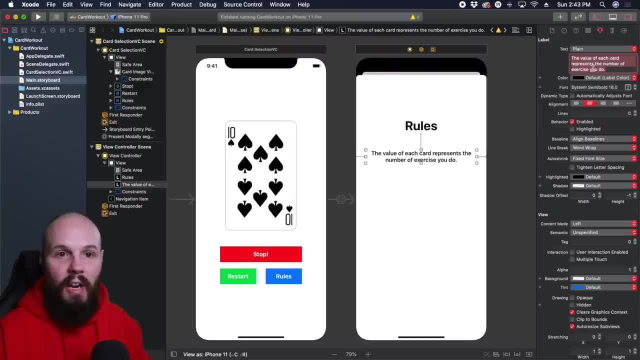 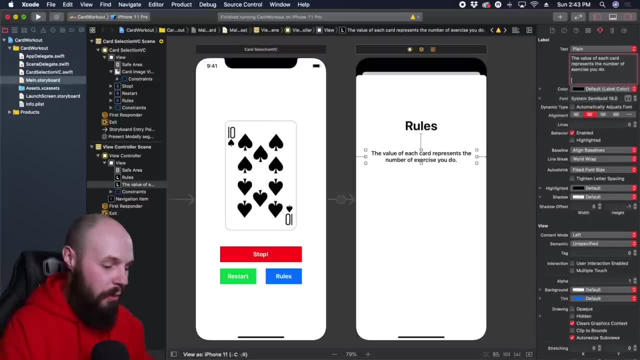 if you click on it Now, when you just hit return, it like enters it. That's fine. But in here, if you hold control and hit return, Now you can have like line spaces in here. So we want one line space and we want to say jack. 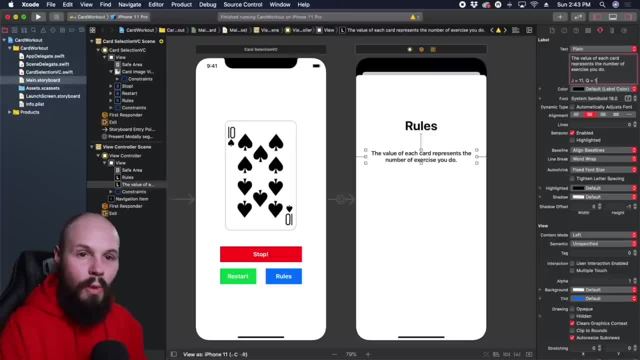 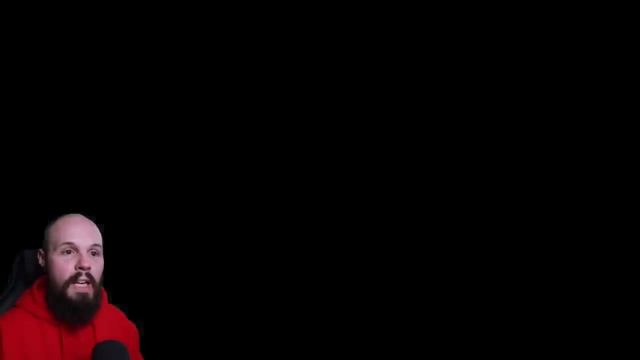 equals 11 comma. space queen equals 12 comma. space king equals 13 comma. space ace equals 14.. Now hit return to enter that And now you can see our label has updated with our rules for our game. So that is our second label, And now we want. 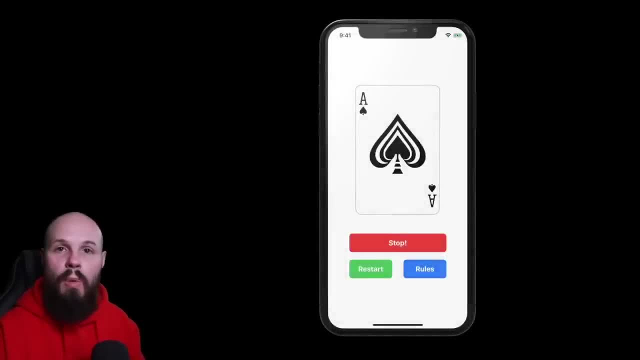 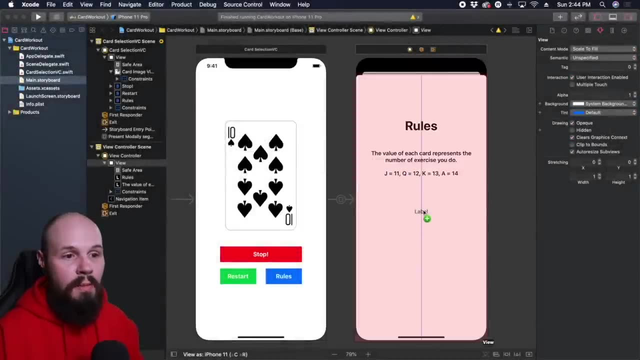 to have, as you can see on our design, this third label that shows the emoji based on the suits on. you know what exercise it represents. So again, plus button, another label right here, And this constraint is going to be a little different. We're not going to pin it to the edges, We're actually 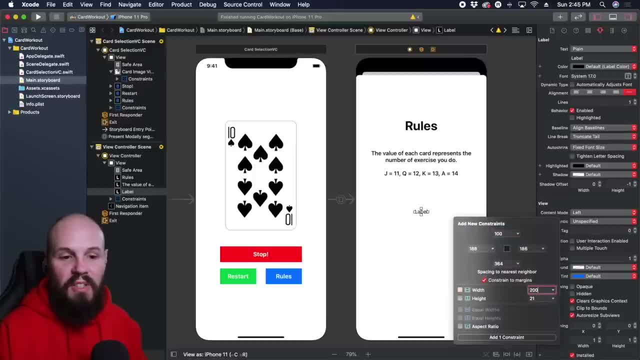 going to give it a hard coded width And it's going to be 200.. And the reason is for design choices on how we want it to line up, Because this label doesn't have to change on screen sizes, Like it's always going to be the. 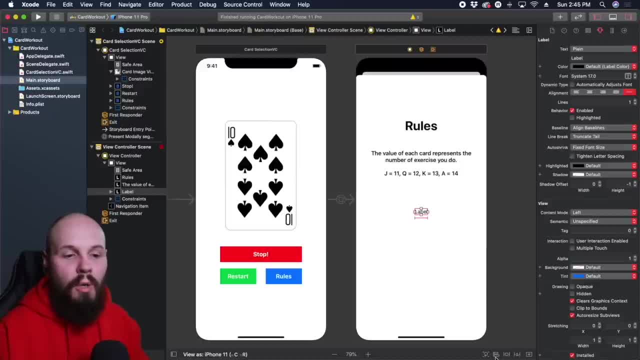 same. So we can do width of 200 horizontally centering container And then we want to pin it to the bottom of our previous label here, The label that says the value of each card represents, as you can see, And we want that to be 75.. 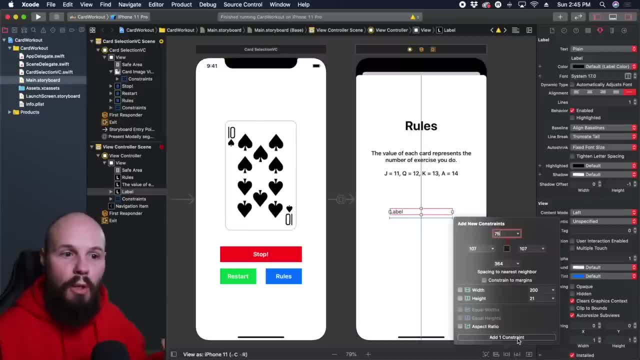 And again how I came up with these numbers. I don't want it to seem like you should automatically know what these numbers are. This was like me building this out previously and tweaking my design. So coming up with these numbers and how it looks is done in the design phase. 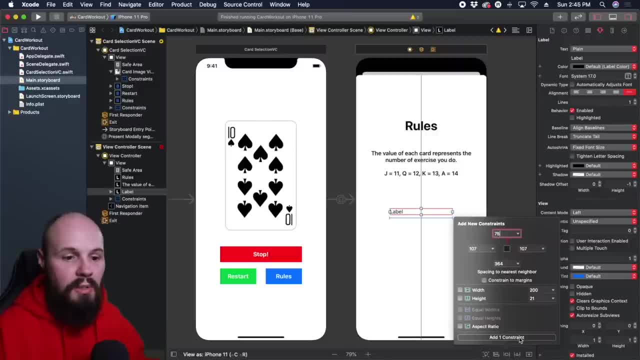 not necessarily the coding phase. That's why I like know these numbers. So add one constraint. So now we need to start filling this with content. So over to our font Again. system font semi bold. We want to make this 21. Hit, done Again these. 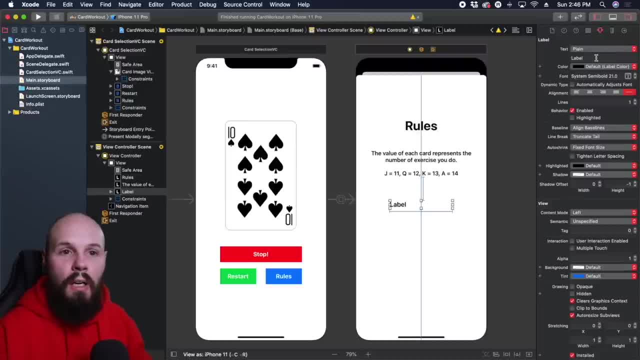 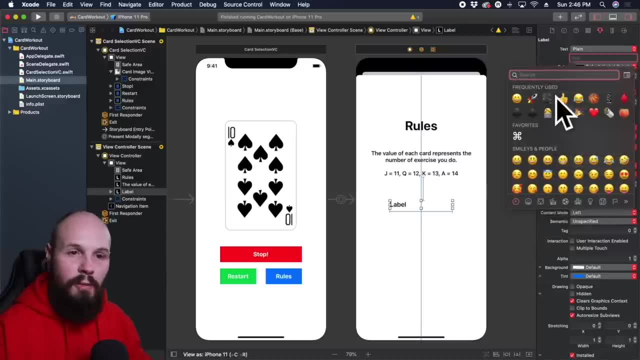 are all things I've dialed in on my design. That's why I know these numbers. Again, let's do command control space to pull up our suits. See, they're frequently used for me. I was building like a poker app as well, and I've built this, So you may have to search. 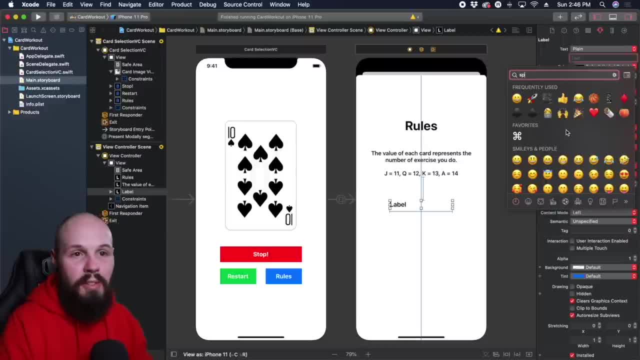 a little bit for these emojis, But just like searching for any emojis, right, you type in spade and you'll see, you'll get the spades. Mine are in my frequently used, so we'll save some time here. So spade is going to. 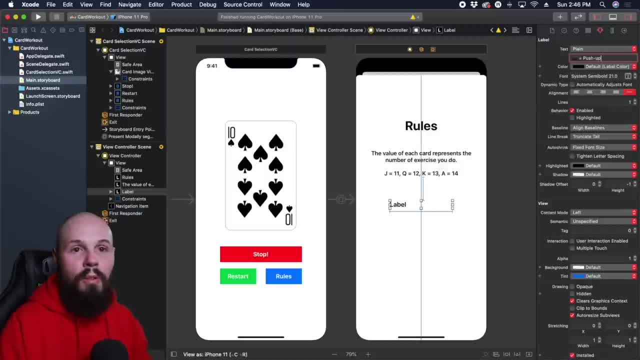 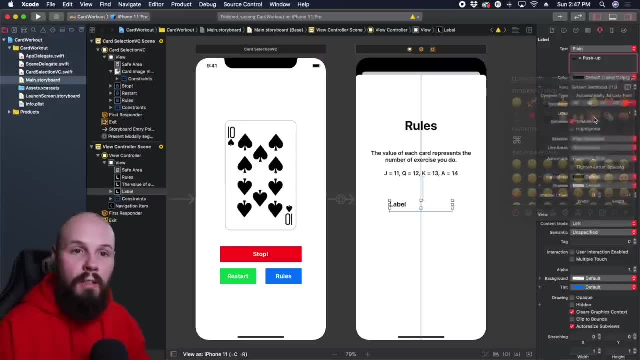 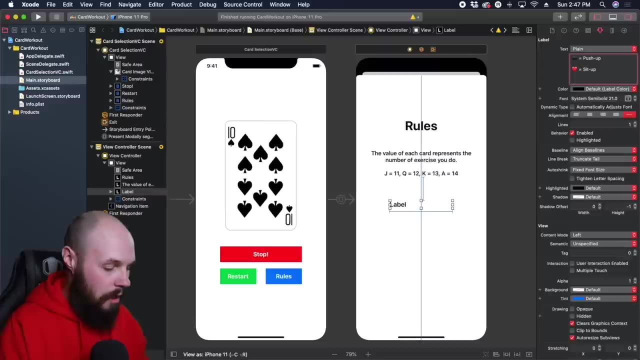 equal: push up, Cool. And then again control return to get those line spaces. Command control space to pull up the emoji. Heart equals sit dash up. It's hard to type with this microphone in my face. And again control return twice Command. 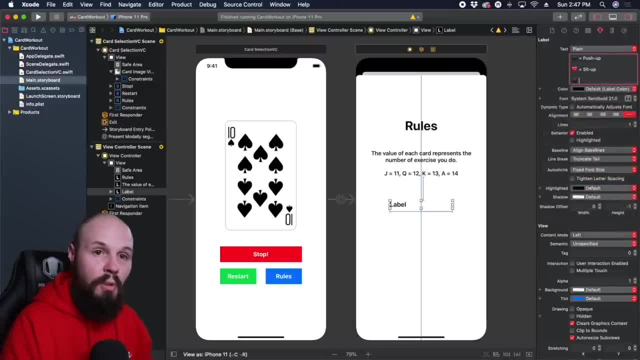 control space for the emojis. Add the club. The club is going to equal burpees And you can fill these in with whatever workout you might want to use. But again, control return twice, Not just regular return. Command control space to pull up the emoji keyboard Super. 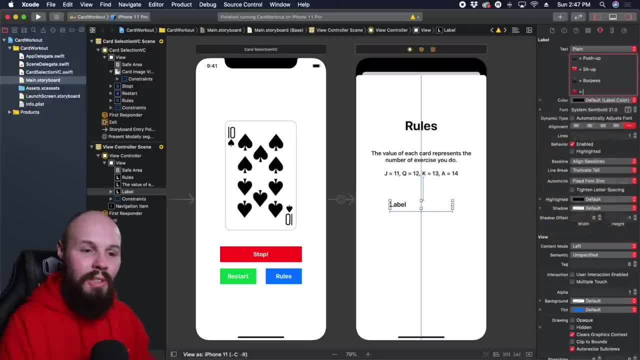 repetitive. I get it. Hit the diamond Equals jumping jacks. Okay, now we can hit return And now you can see our label is here, but we're only seeing push ups And then, just like this previous label here. number of lines we have to set. 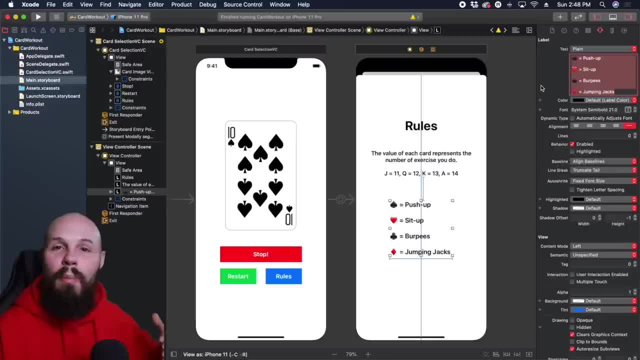 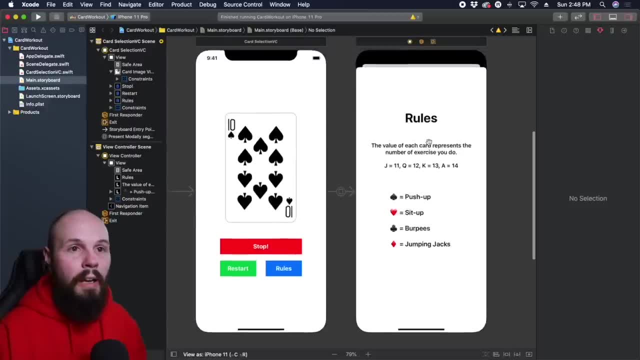 to zero. There you go. That'll make it adapt automatically to however many lines you have. And again, that's the labels. It's called intrinsic content size. So that's all we have to do to set up this screen laying out the UI. Maybe you notice something. 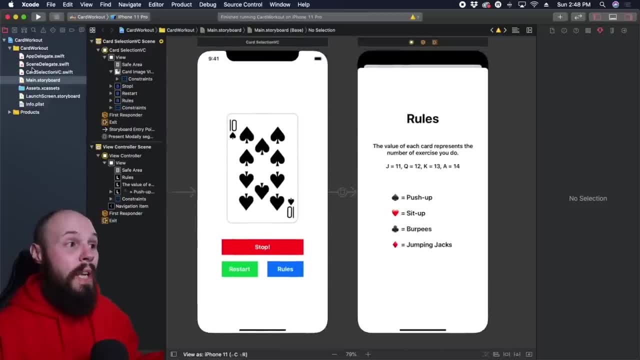 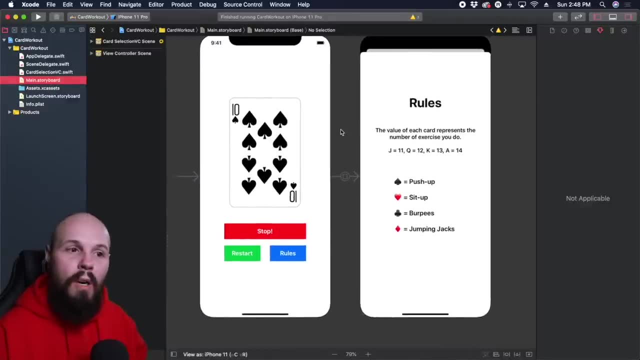 You notice how on this card selection vc we have code, So we had to actually create a card selection vc for that code. Well, we can lay this simple rule sheet out on storyboard, Right? There's no logic going on, There's no interactivity. We're just showing a simple 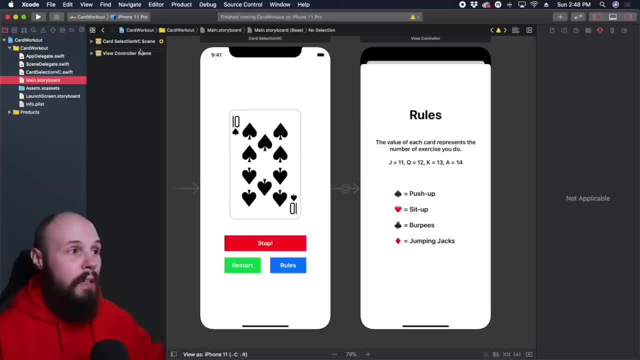 rule sheet and then sliding it down, So we don't even need to create a view controller file to have the code. So again back to the pros and cons of like doing everything in code and storyboard And, how I said, like for super simple screens. 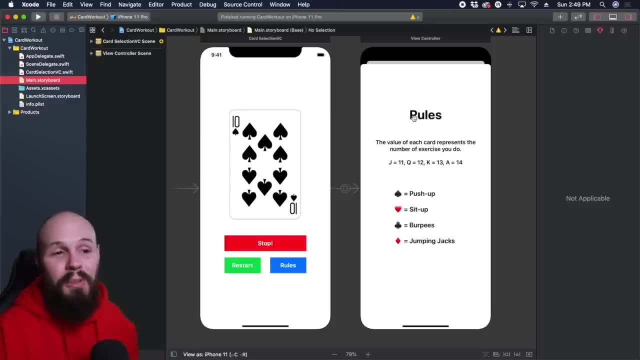 I prefer storyboard Because, again, this is one of those super simple screens or there's no logic. You're just showing the rules, No code at all, Just 100% on the storyboard. Very, very simple. You don't clutter up all your code Again. 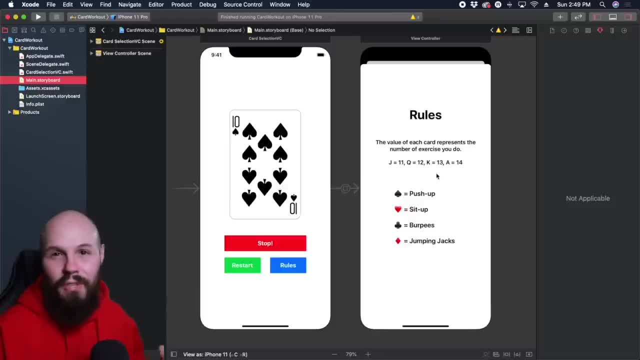 that is just one of the advantages of storyboards. There's plenty of pros and cons for both, But again, I'm trying to illustrate those to you so you can get experience with it and start forming your own opinion. So let's run this to wrap up this video. 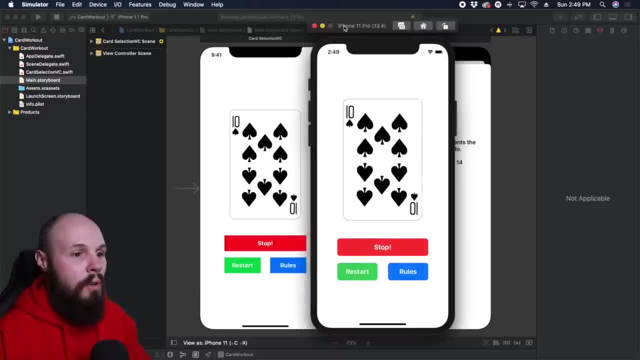 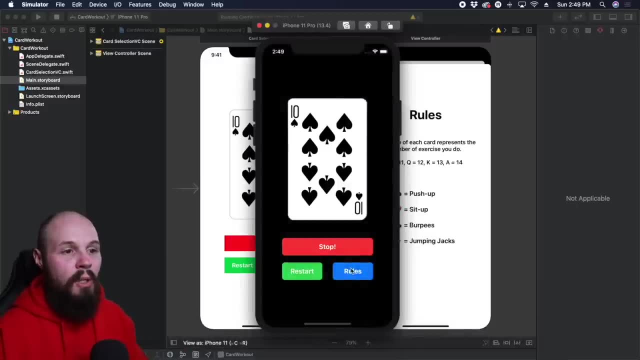 And things should be working nicely. So here's our phone. Hit rules: Pulls up the rule sheet. You can slide it down. Do the old command shift A. Get into dark mode. Bam, Looks good in dark mode. Tap rules. There you go. 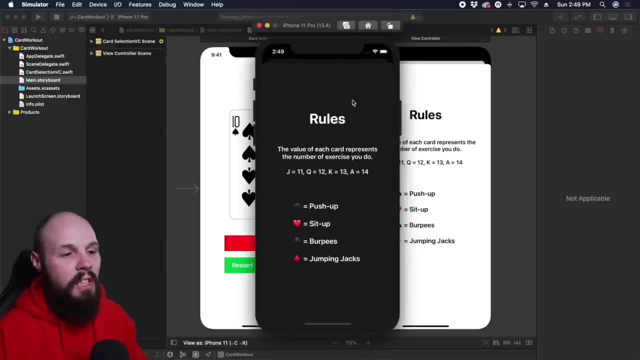 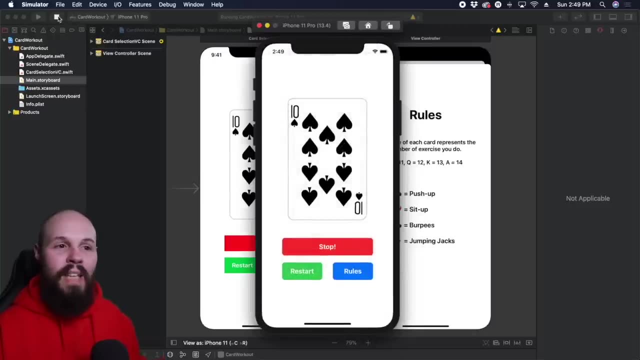 You get that nice dark gray looking color for the modal sheet. Slide it down, Command shift A Back to light mode Rules. There we go. So our general UI and navigation is laid out. In the next video we're going to start working on the 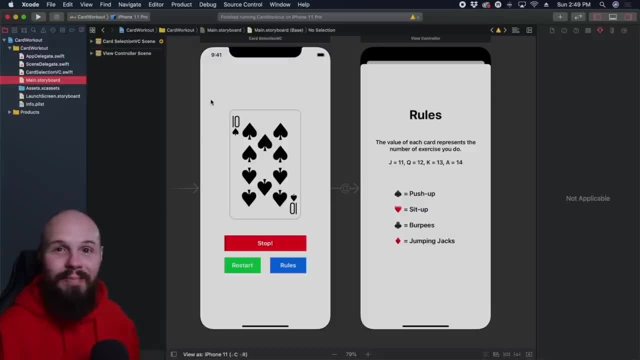 logic to actually make this app work. Alright, Let's do it. Here. we are Right where we left off. Now the only thing that's left for this app is to set up our timer, So we constantly change this card view to cycle through all the cards. 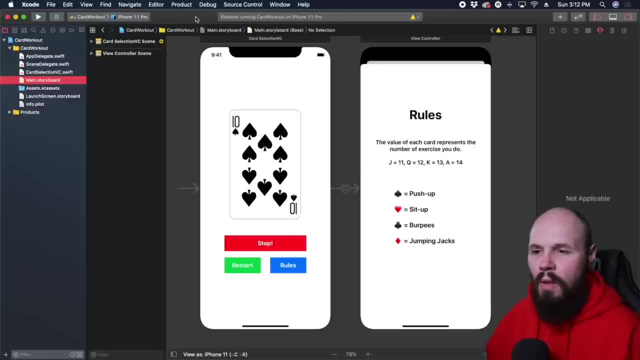 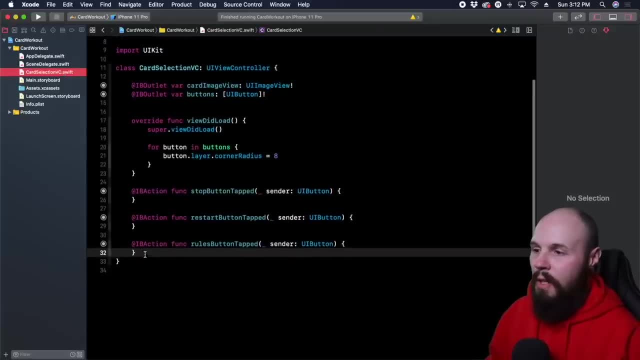 To do that, we need to create our array of cards as well, And then implement the button functionalities. So let's go to our code here: The card selection VC. As you can see, we already have our button actions ready. Let's start by creating our timer. 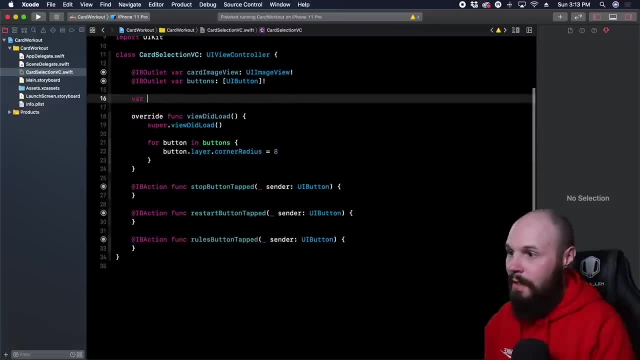 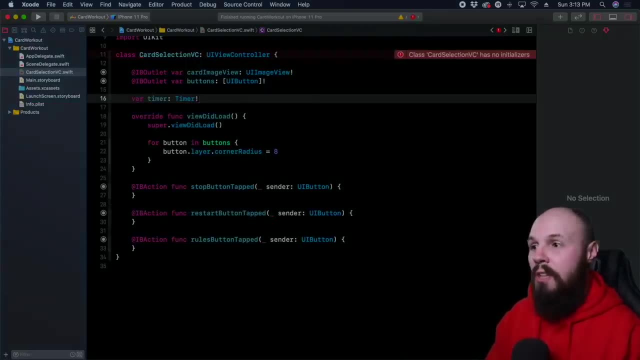 So up here under our variables here we'll do var timer of type timer and then we're going to implicitly unwrap this. This is what this means. So remember, we did this before with the color variable in the color table view app, But we left that. 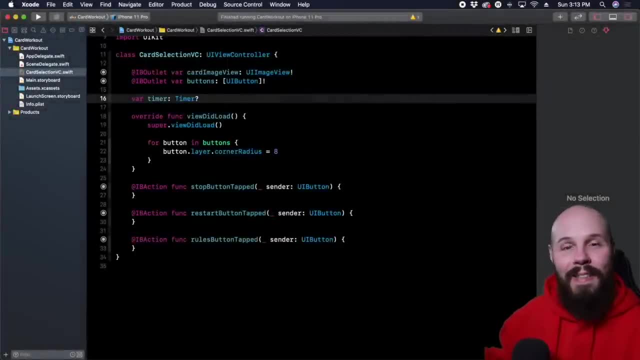 as an optional. We left that as a question mark Because, remember, we were passing the data. That view controller didn't always have that data. It was relying on another view controller to pass it that color. Well, here, with this timer, we're going. 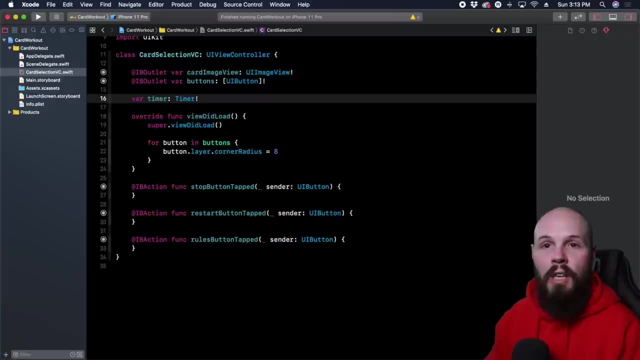 to initialize this timer right away. It's contained within here. So, again, you're going to get various opinions on force unwrapping. In my opinion, this is one of the times where force unwrapping is fine, So we're going to do that. 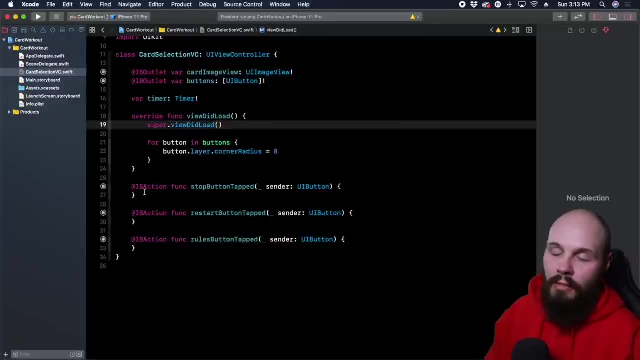 And again, that is because here in view to load- Well, actually in another function that'll get called in view to load- We're going to be initializing that timer and starting it. We're not relying on a network call or another view controller to pass us that. 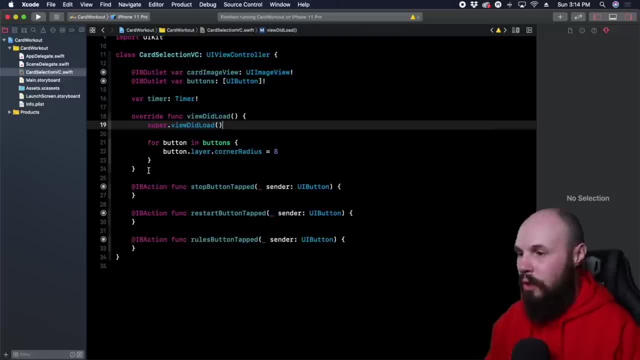 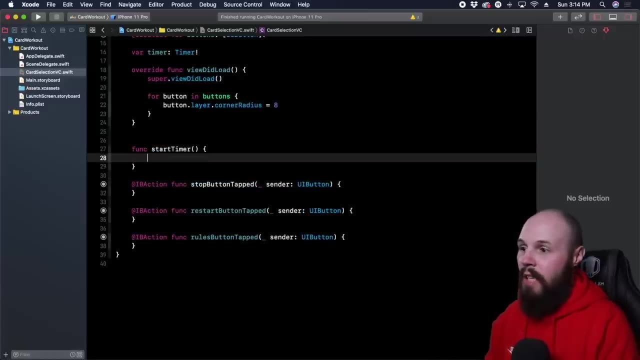 data. It's all self contained in this view controller. So here below view to load, let's write a function called func start timer And here we can do timer equals. so this is like I said, we're initializing our timer here: Timer dot- scheduled. 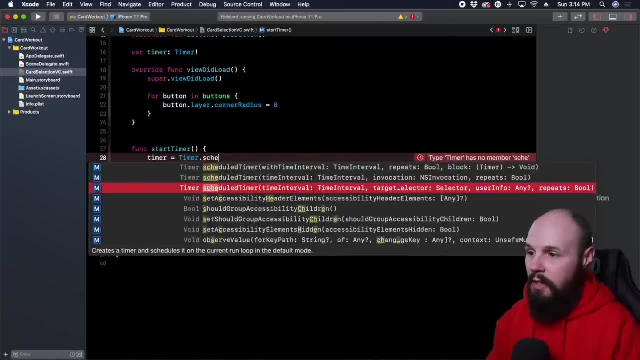 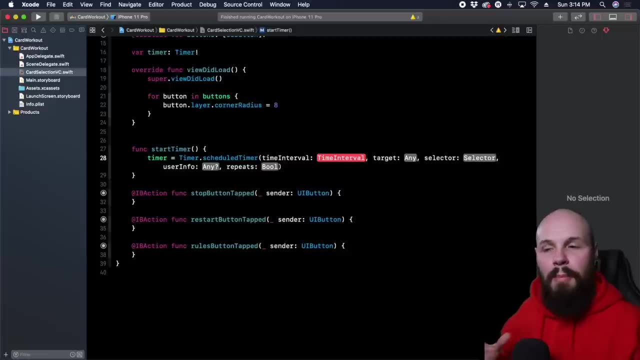 timer here And we want to pick the one that has the selector here. that you can see is the third one down. So time interval: This is how often this function fires off. Let me back up a big picture and explain what the timer is actually doing. So we set our time interval. 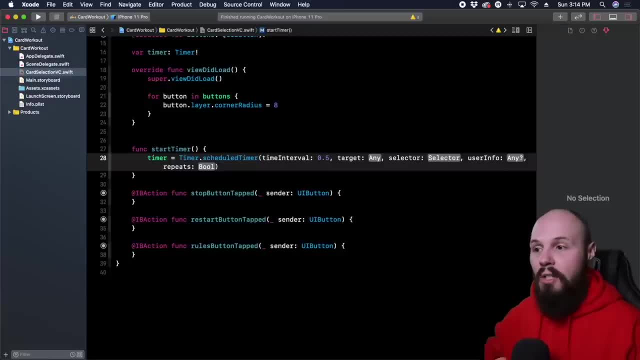 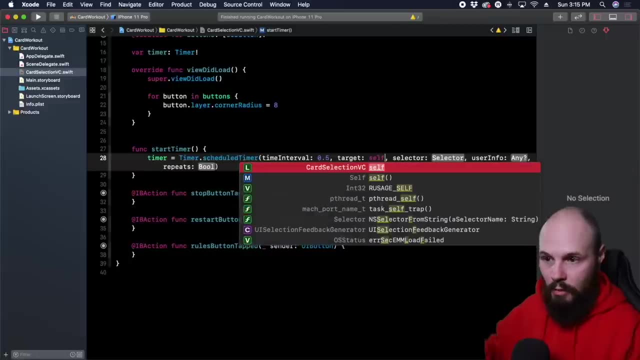 so let's say 0.5 seconds, Right, Half a second. So every half a second this timer fires off and it does something. We have to tell it what to do. So real quick, the target is self. that's our view. controller. 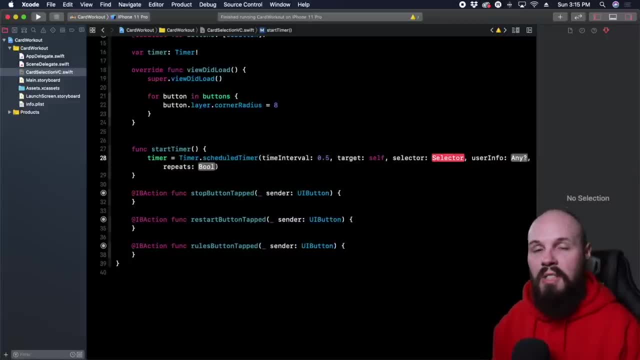 Selector. Okay, So this is what is firing off. So the selector is where you pass in a function. So you have to do hashtag selector and you can see it takes in an at objc method. This is a little bit where we're interacting with objective C. 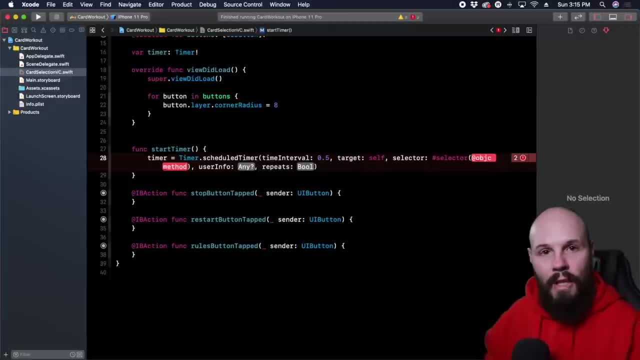 at a lower level, Like we don't have to do anything with objective C, but at a lower level we're interacting with an objective C functionality. Let me get rid of this write pane here so it looks neater. So let's write this function that we're. 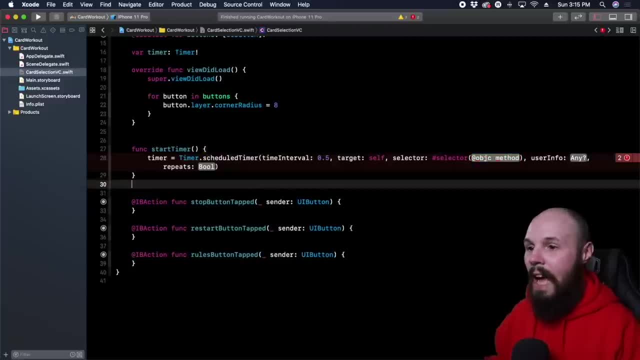 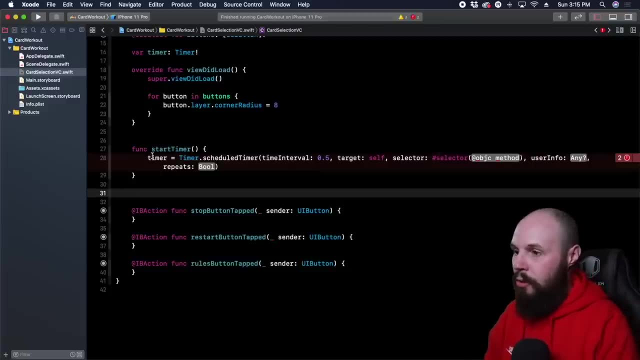 going to have to pass in So at every half second. what function do we want to fire off? We want to change the card that is showing in our image view. So here we'll do func, show random image, right, And then that's where we're going to write. 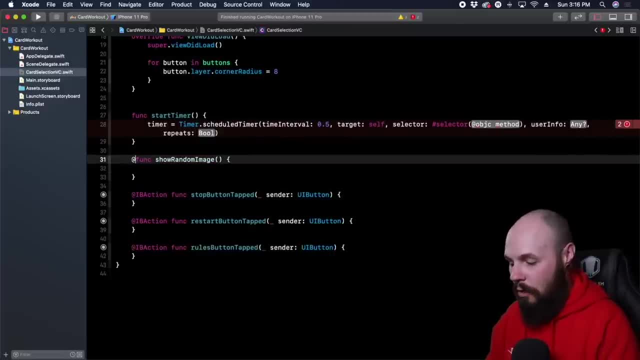 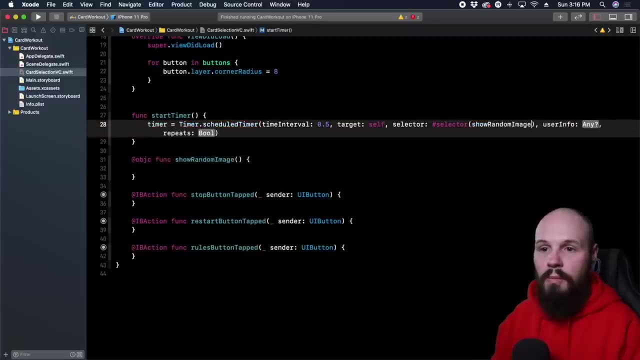 that functionality. But remember, this function has to be at objc, right? That's what you see here at objc method. So now if I pass that in show random image, I don't know why it was a strike through- We'll do a command B to make sure we get all of our auto complete. 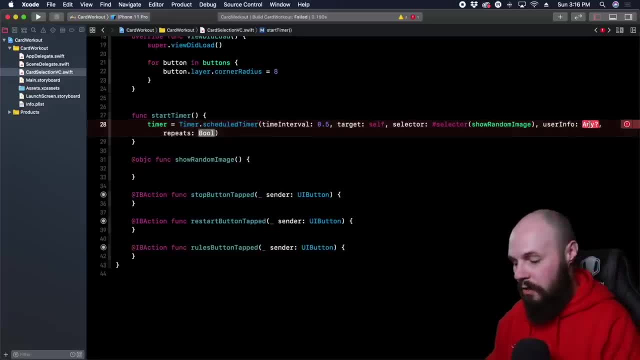 and everything. It's yelling at me because we haven't totally finished this, so let's do that. So this is nil for user info. We're not passing any info to our timer And then repeat: This is big. You want to set that to true? You can see it takes in a. 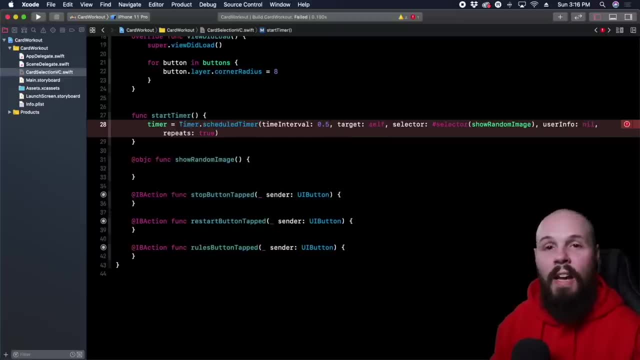 boolean. So make that true, Because, again, we want to run this timer every half second. You can also create a timer that doesn't repeat, So you want to say maybe, hey, after 20 seconds on this screen, show an alert. That would be something that only runs once. 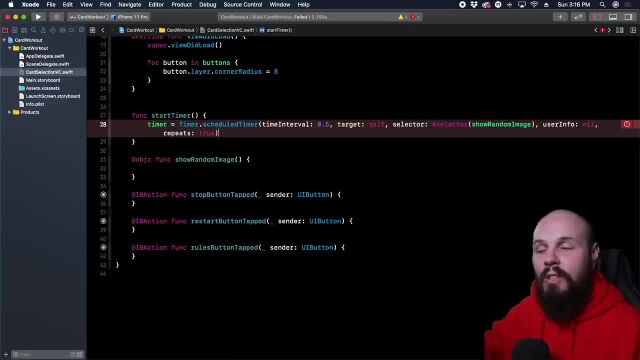 Because we're constantly changing our image. we want this to run repeatedly, So that's why we're putting it to repeat And do command B so we get rid of that error. Yep, we got rid of it. So sometimes, if an error is not disappearing, 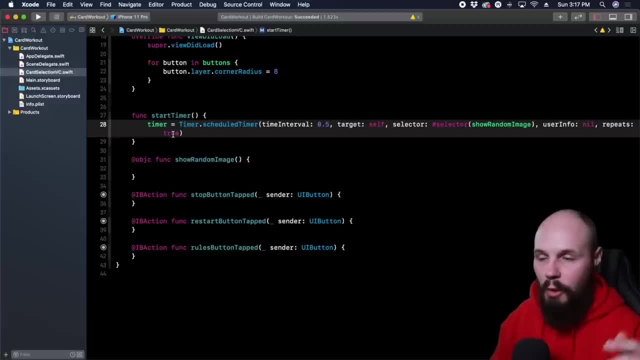 after you fix it, do a quick command B to build your project and that'll build it and you should get rid of any errors. So here we have our timer again. Every half second the function show random image is going to fire. Right now it's not doing anything. 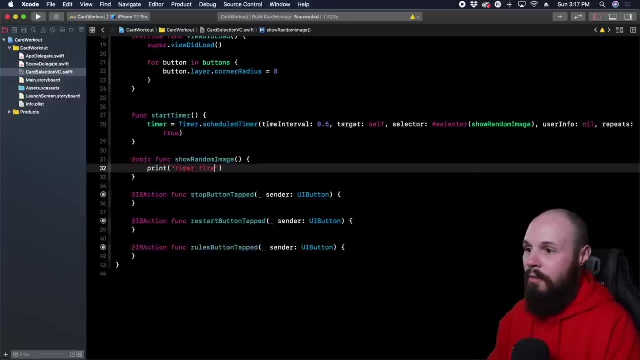 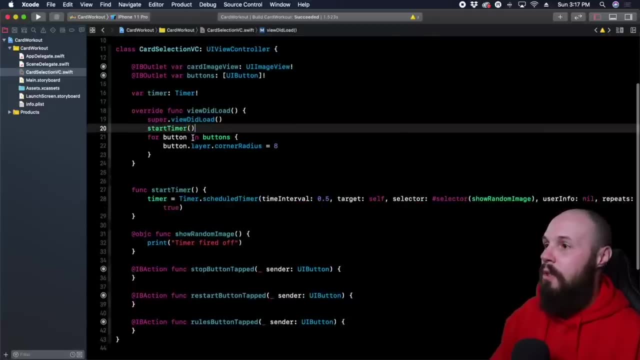 But we can test it. So print timer fired off, Right, and then make sure we actually call this start timer function here. So start timer. So let's run this to test it and we should see in our console just a bunch of print statements firing off every half second. 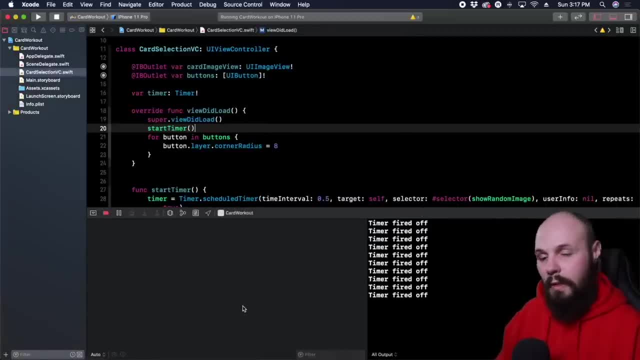 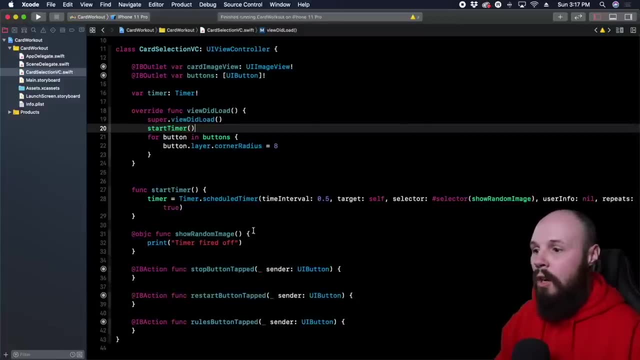 Yep, you can see it right here: Timer fired off. Timer fired off. Timer fired off, So our timer is working. Now we just need to, instead of printing something, we need to change the card image view. So we can do, you know. card image view. 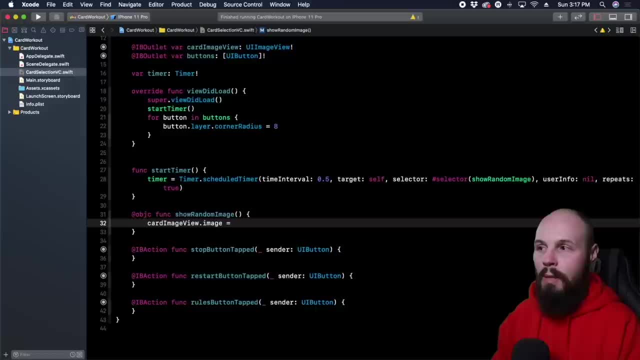 dot image equals. well, we need the images. Remember, we brought all these in. I'm actually going to delete this line of code so I can get rid of this error. So let's create an array of card images, Right? so that way we can just pull a random element from. 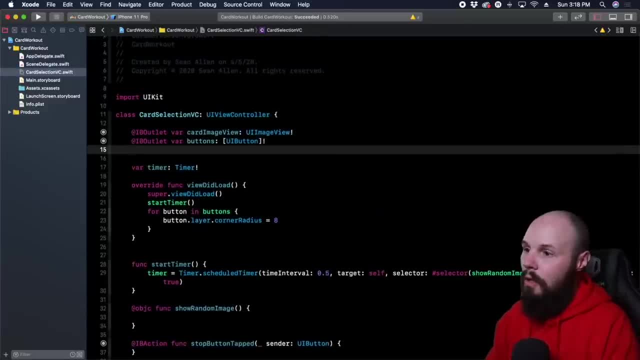 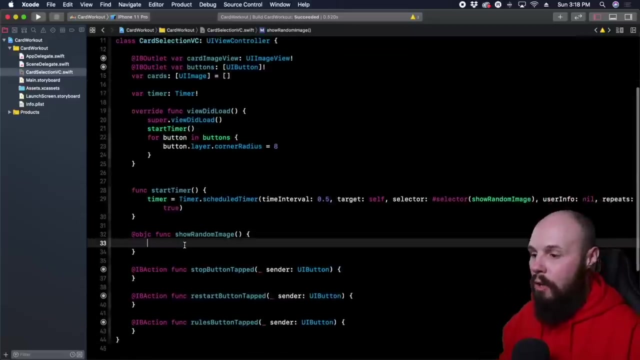 the array. So let's go up here and do var cards, which is an array of UI image image here- and that is going to equal an empty array. Right now it's empty because we'll populate its images for now, but I want to finish up this code right here, So 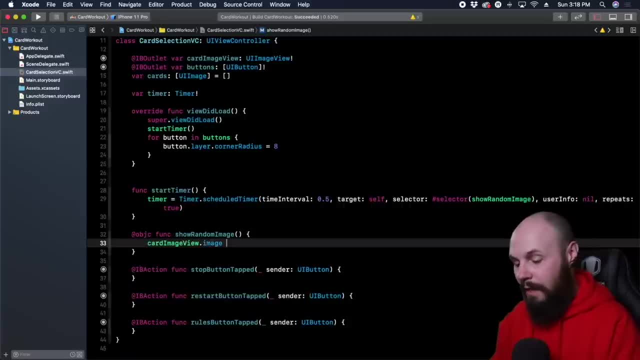 we can do: card image view. dot image equals cards. dot- random element. So what this is going to do is this is going to pull out a random element from the array. Now you'll notice this is an optional. Hopefully this is a review. Why is this an optional? 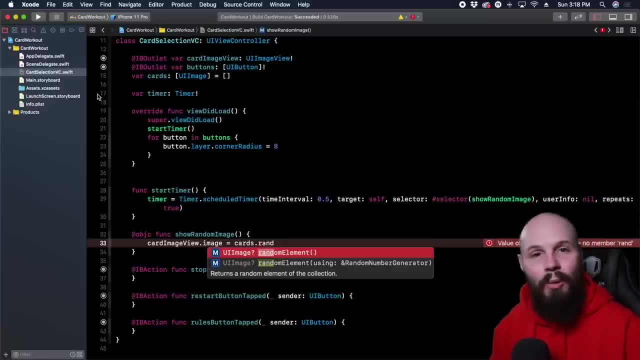 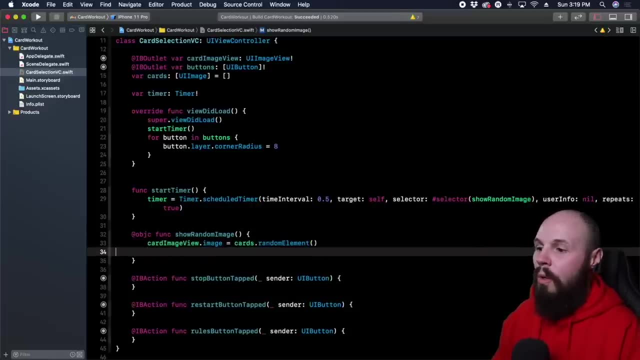 Because our cards array could be empty and you can't pull out a random element from an empty array, So we can hit return Again. there's multiple ways to unwrap an optional, So what we're going to do is just give this a UI image. 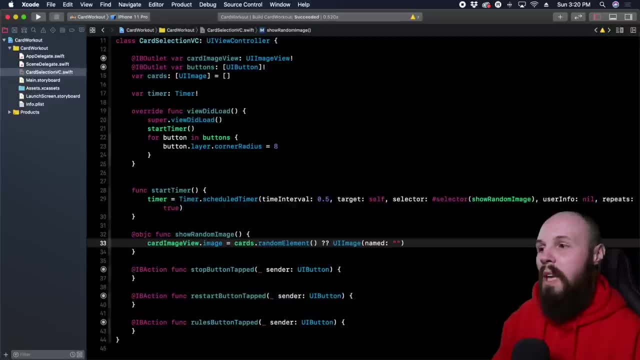 named and we're going to pass in a string and we want the ace of spades. That's going to be like our default image should this thing break Again. that way it doesn't crash if there's like an empty array. So back to my assets here. 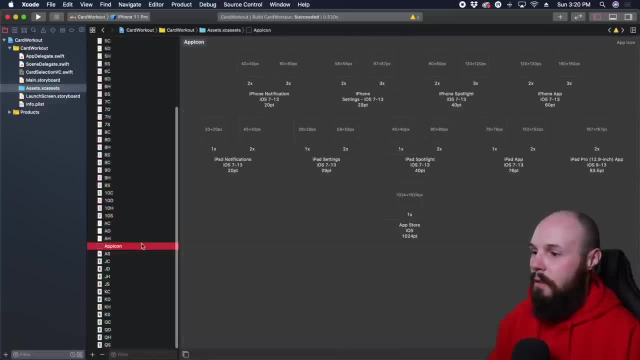 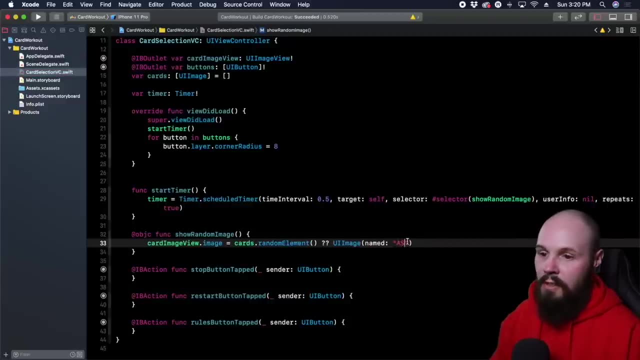 I can see the ace of spades right here. Click everything. there you go, Ace of spades. right, there is just the string AS. Right, so go back to our card selection and named AS. So this way, if the array is empty for some reason, which is empty right now- 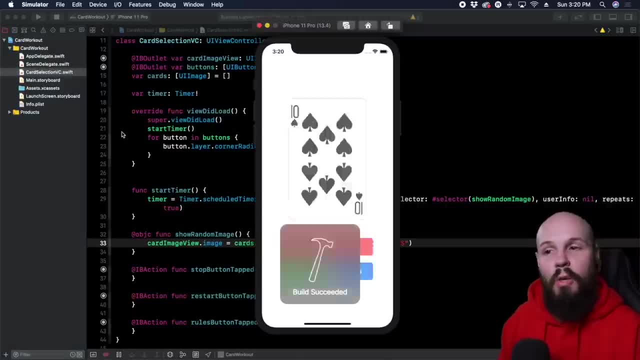 actually let's do this. So this is going to constantly remember. the ten of spades showed up in the beginning. well, there you saw. it switched to the ace of spades because that array is empty and that's like our default. like, don't crash our app. 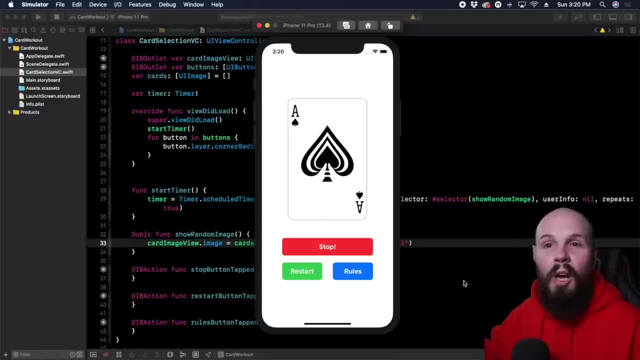 just show the ace of spades. Now, if you were really building a user product, maybe you'd want to like show a joker and say, hey, the cards are empty. something happened like a fun little empty error state Again. for now we're just going to show the. 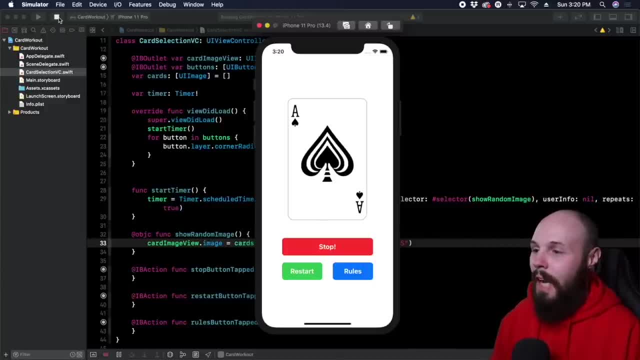 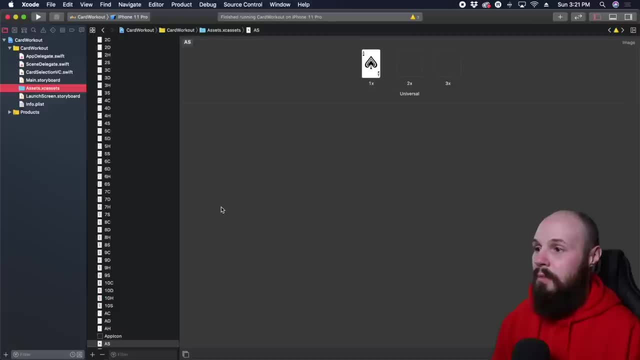 ace of spades as our default. So stop that. our timer seems to be working, but we need to create our cards here like an array of cards. So, as you saw right, there is 52 cards in a deck, right? so that's a lot. 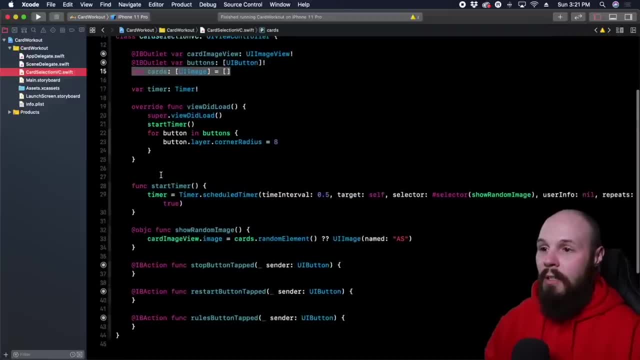 What I'm going to do, instead of creating that array here and really getting this all muddied up with this data- right, because this array of cards is essentially data that we're going to use- I want to get that out of the view controller so it doesn't clutter up my code. So 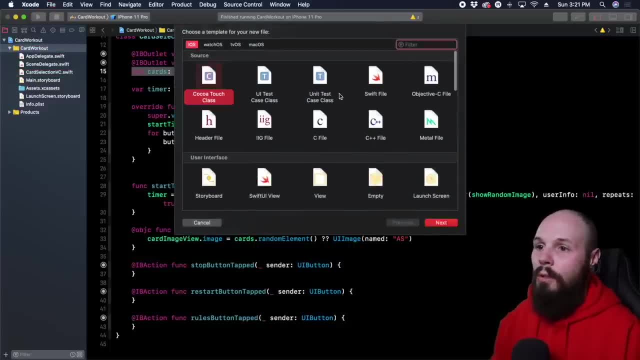 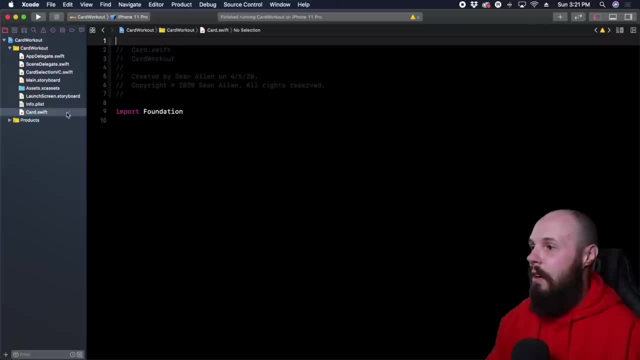 on the file of card workout. do command n: do a new swift file. just blank. hit next. we're going to name this card, hit create. so now we have a file called card that we're going to put up here and it's kind of like a data model, if you. 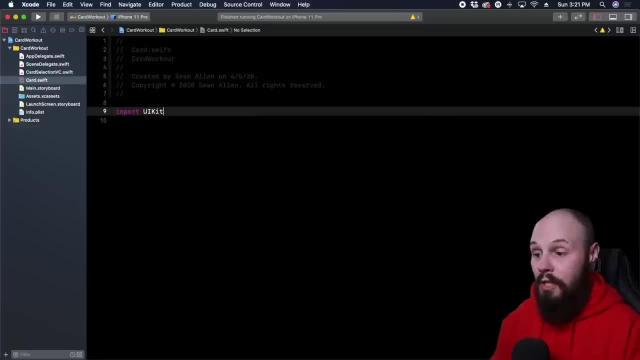 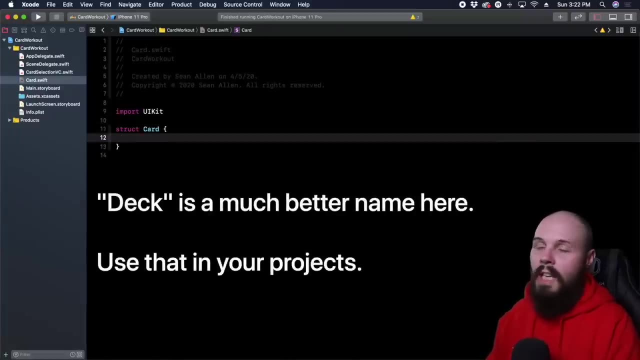 will and we need to import UI kit because we are going to be using UI image views here or not. image views images, so here I can create a struct called card and on this struct I can have a variable. so I can do static var, and we'll explain why. 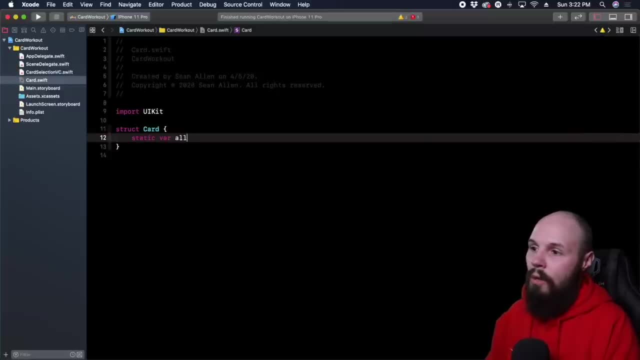 I did static here and I'll show you in a second, but I can do all values and that is going to equal and I'm going to fill in this array here and I'm going to do this on multiple lines because, as you can see, this is going to be. 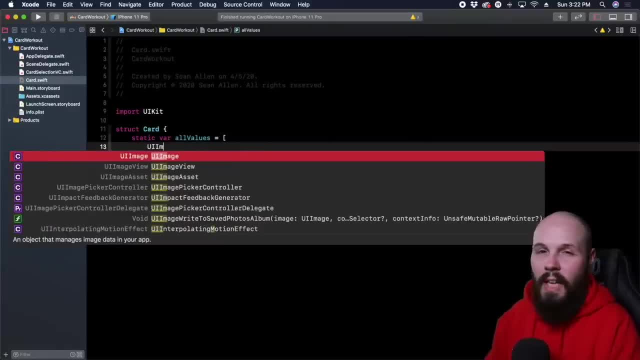 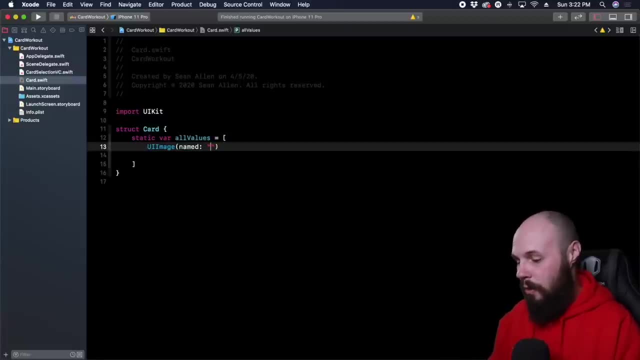 a lot. so we're going to do UI image. I always forget the second i in UI image. I always do that UI image. same thing we did with ace of spades named. and we're going to do two of hearts right 2h and again, if we go back to our 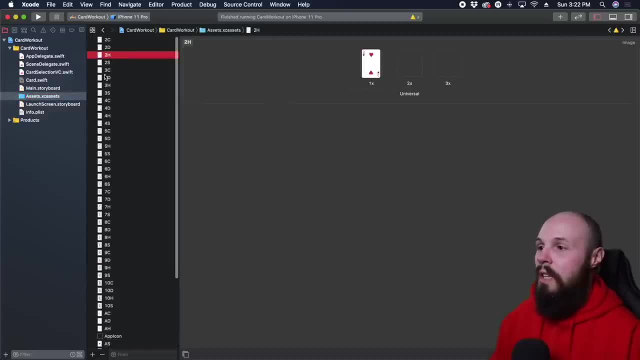 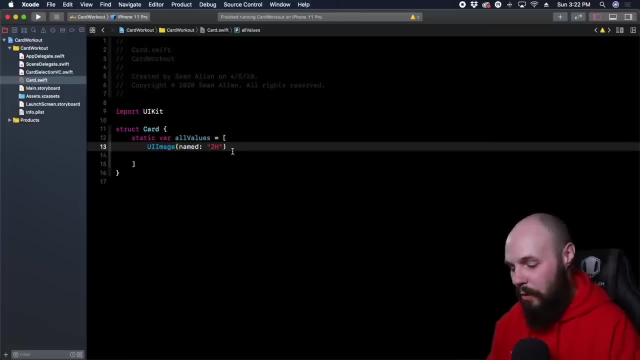 assets. here you go, you see 2h. there's the two of hearts, and they're all named like that, right, like so, the four of clubs is 4c, so that allows us to create this pretty quickly, actually. so 2h, and we're going to create our array. well, 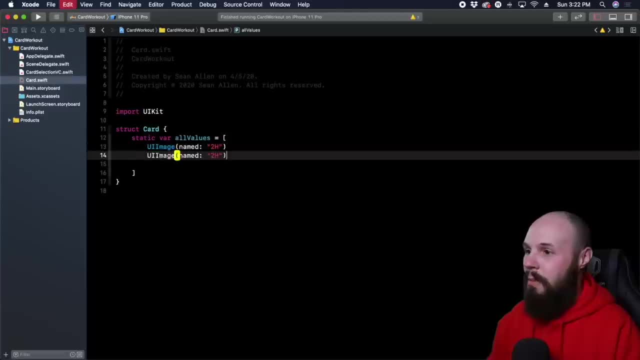 I'm going to do this. I'm going to do copy: paste, paste, paste, paste, paste, paste. we'll see here. you'll see how quickly I can do this here. so this needs to be commas after all this. so watch, if I hold option and drag down, now I get all. 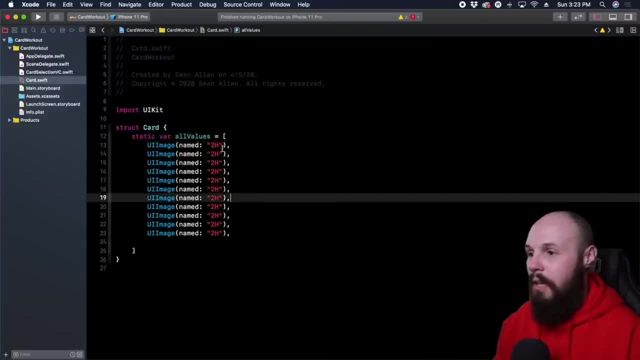 these cursors so I can just do comma. there you go all that. now you can see again hold option. well, that'll come later. I actually have to do this manually, I think so two, two of hearts, three of hearts, four of hearts, five of hearts, six of hearts. you'll see, I'm not going to have to do this for the 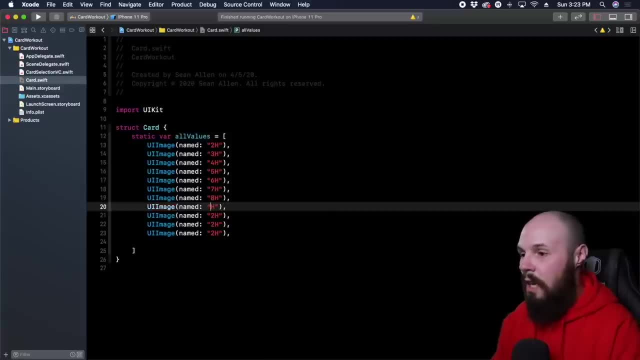 whole deck. I can do some nice copying and paste and batch changing features here. nine of hearts, ten of hearts, and then we get jack of jack of hearts, queen of hearts, and then I need two more here. so command c, king of hearts, ace of hearts, right? so 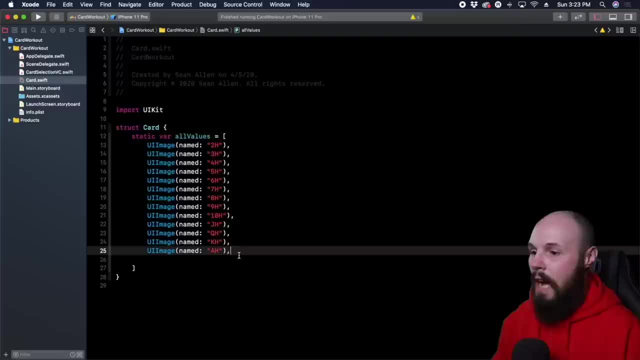 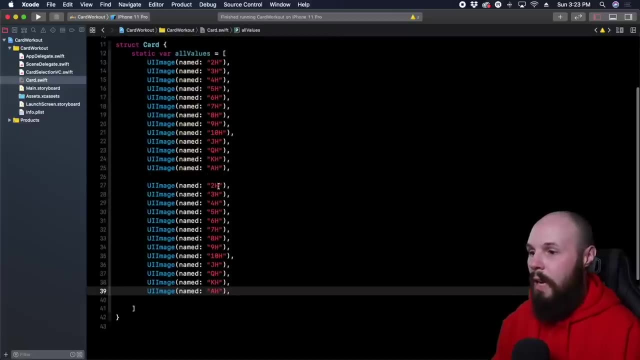 kh. ah, okay, so now I'm going to copy and paste this whole thing. so there's my hearts, right, so copy. now let's do spades. so now what I can do is again hold down option, highlight all these h's. uh, kind of sucks, because the ten of hearts messes it. 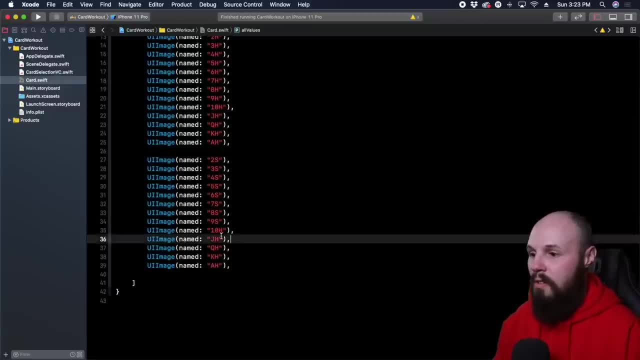 up, but highlight all the h's. put a capital s there. cool, there's my spades. just change this ten. that's messing me up. and then, option uh, highlight those h's, make them spades. boom, there's my spades. we're done. rinse and repeat. 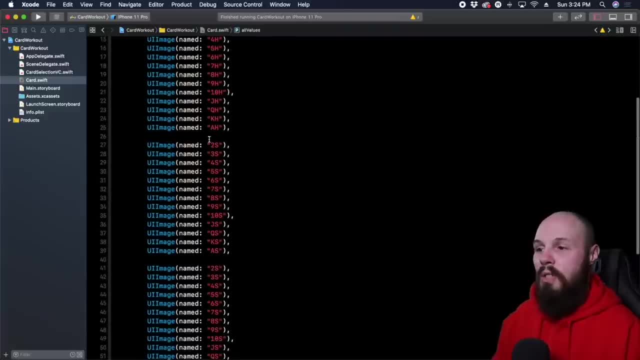 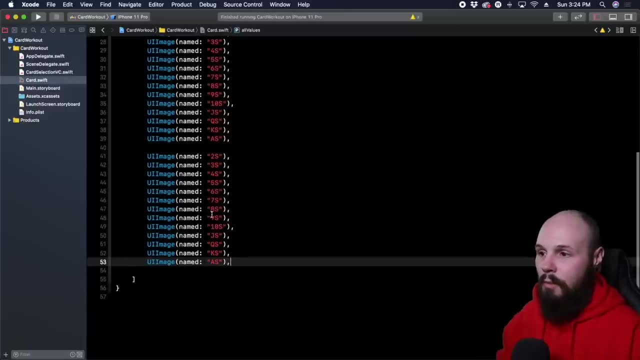 for, uh, clubs and diamonds. and you see, I'm putting this extra space in here. this is just to visually separate, like. so I know, like, hey, these are all my hearts, these are all my spades, uh, these are all my well, they're going to be clubs. 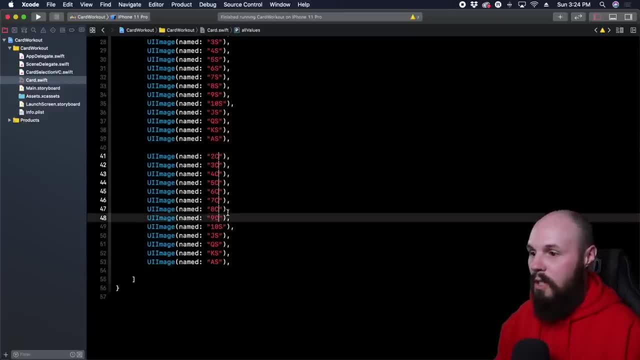 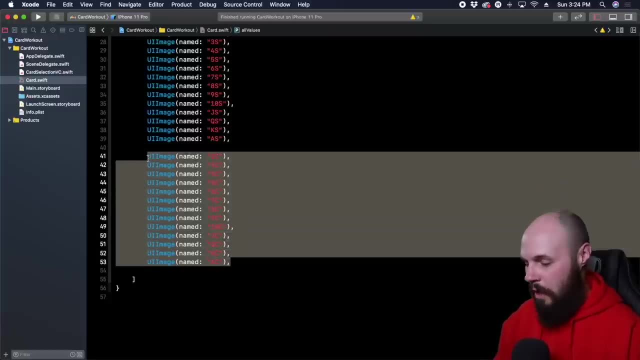 but um, that's just an optional way that you can add some space in there. so change that to a c for clubs. this is a c for clubs. again, hold option: highlight c for clubs. cool, do the same thing for diamonds, and we're done. so copy paste: hold. 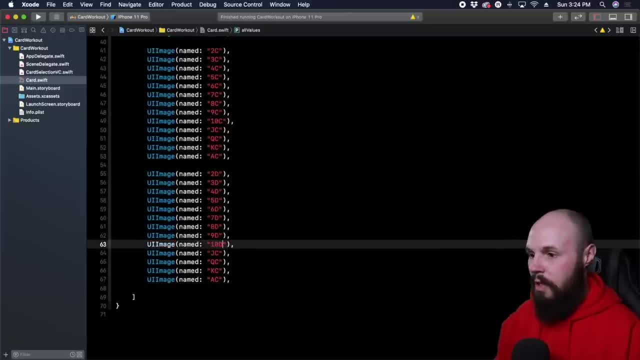 option highlight them all d, change that to a d and option all that. oop, nope slipped on the option highlight there, uh, d. so there we go, uh. so there's my array of all 52 cards: uh based image. I don't need the comma for the last one. and one thing you may have: 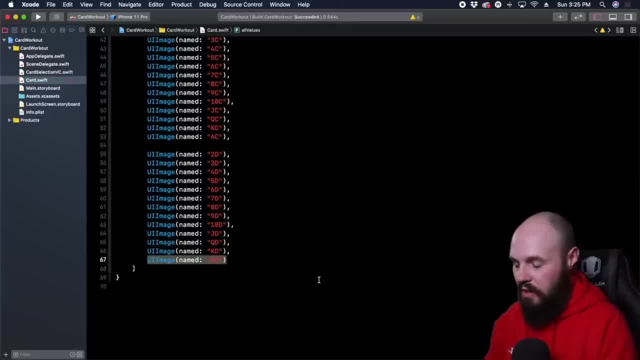 noticed. let me actually retype this last one. so, and it's ad. uh, so you see diamonds ui image named and you see it's an optional, so all images are optional. uh, that would be in case you for some reason deleted, uh, the images from your project. so, uh, again this. 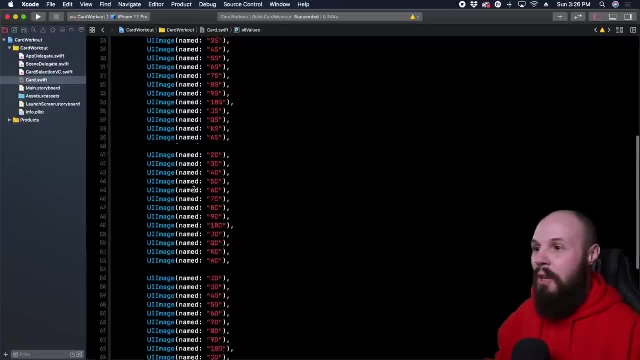 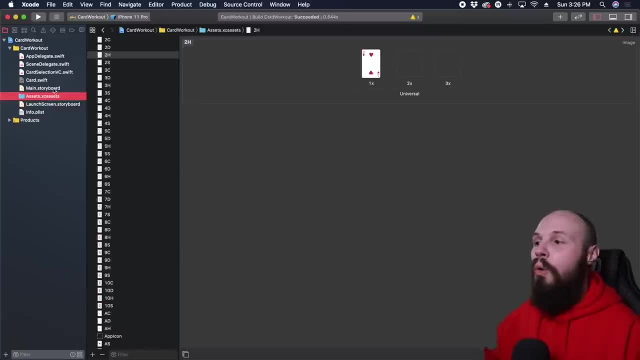 is where you're going to see force and wrapping used. right, because we know these images are in our app. right, they're. they're downloaded to our app like they're in our project. we're not. you know, if you were downloading these images from a server and you could have network. 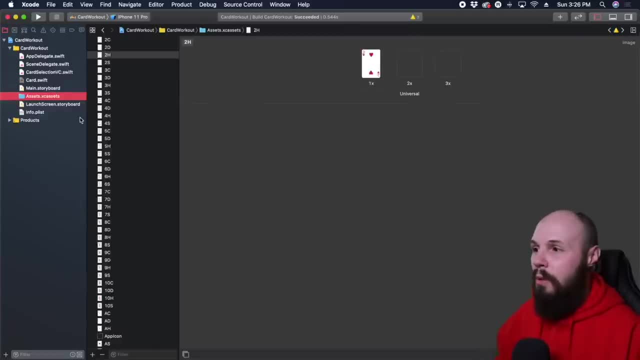 issues. you know something could go wrong. of course, you don't want these to be optional, but because these are like built into our app assets within our app. again, my opinion is this is the time when force unwrapping is okay. now, of course, there are always caveats. 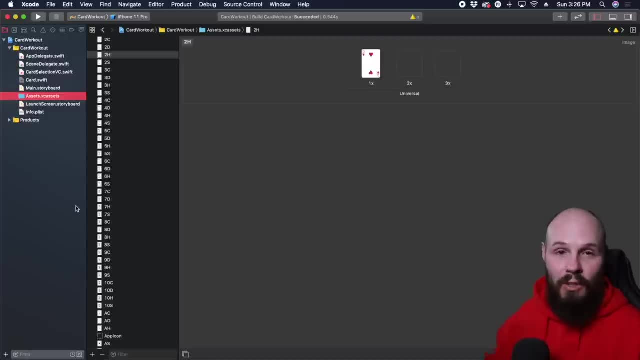 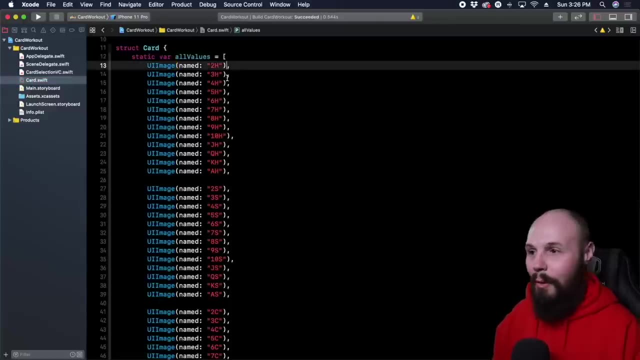 right, if somebody were to come in and delete all these assets, then our app is going to start crashing. but yeah, that's what I think of that. so, uh, because, again, the proper way to do this would be to, like you know, unwrap all these optionals. uh, but we're. 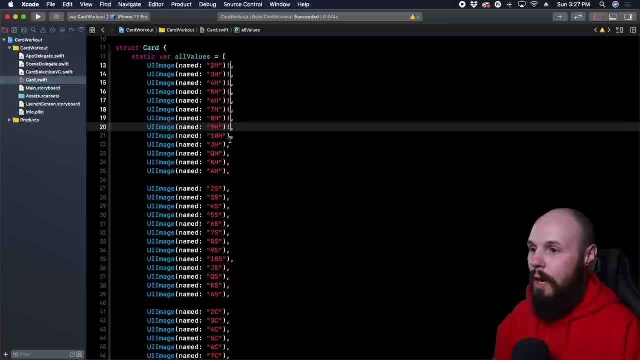 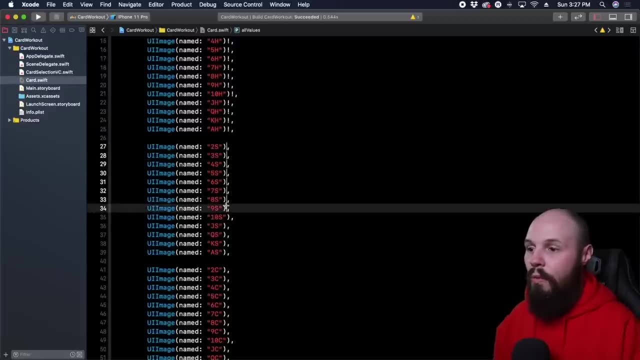 going to hold option, just like we did before, and do mass force unwrap here, one there, again and again. I want to be very clear that you will hear some developers, uh, that say that no force unwrapping, ever, never do this and technically, like I said, they're, they're not by the textbook. 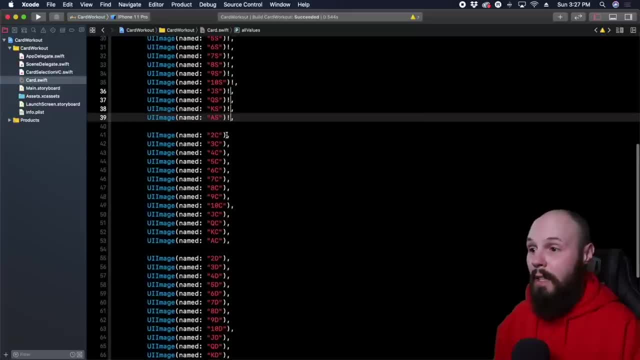 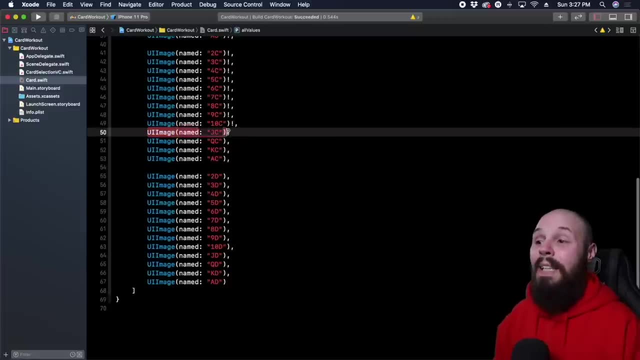 you're not a hundred percent wrong. um, here's my take on it. and again, programming: what you're you'll find over your time in this space is that programming is highly opinionated oftentimes. I saw a tweet the other day that says: you know, we have a million different ways that we can. 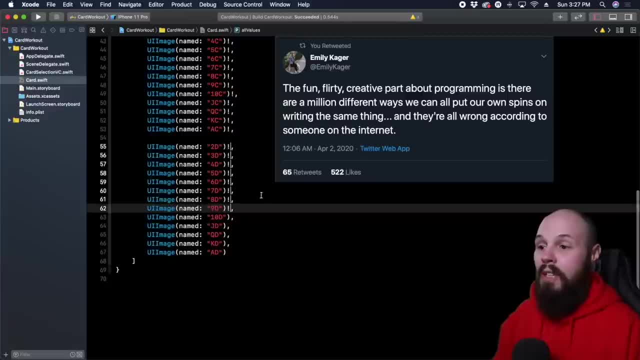 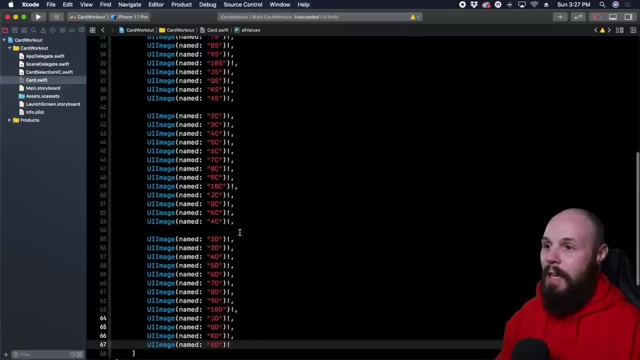 all write the same thing and get the same results, and every single one of those ways is wrong, according to somebody on the internet. so, uh, yeah. so again, I guarantee you there's people that disagree with what I'm doing right now, but my reasoning and this is: this is the thing, as long as you know. 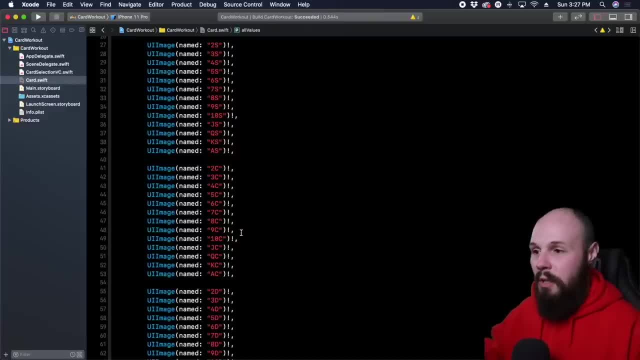 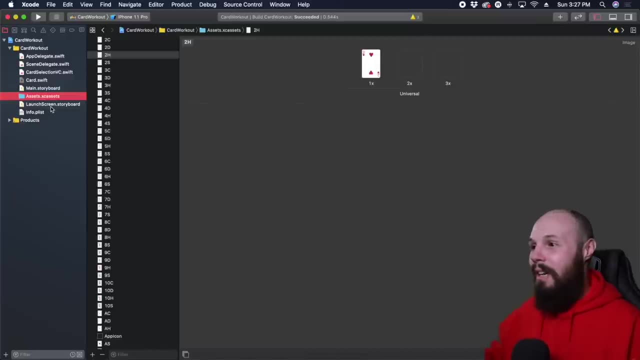 why you're doing it and the consequences. then you can make an informed decision again. the reason I'm force unwrapping these is because I know these are in my project. right, I'm not downloading these images. they're going to be there unless somebody comes in and sabotages my project. 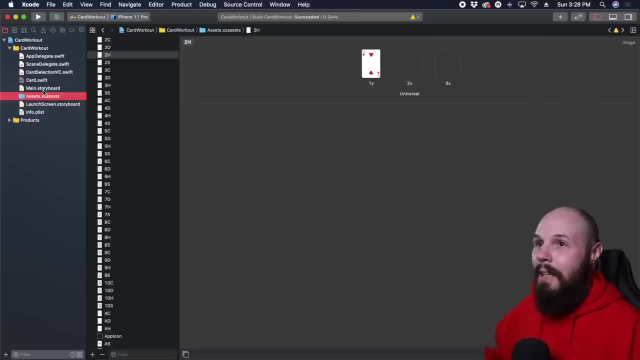 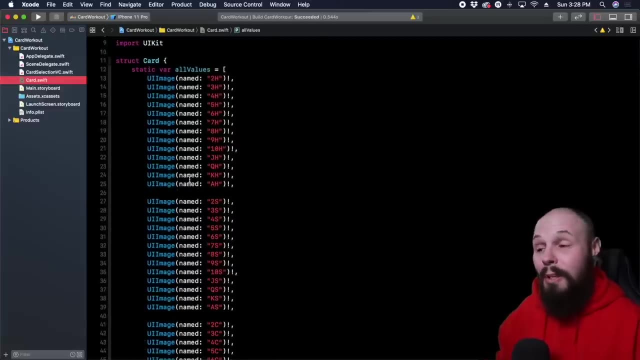 and deletes the image. so, uh, but again, like I said, that's why they're technically correct to force unwrap these. or I'm sorry to not force unwrap these, because it is possible for somebody to come in and delete the images, but you've seen what it takes to unwrap. 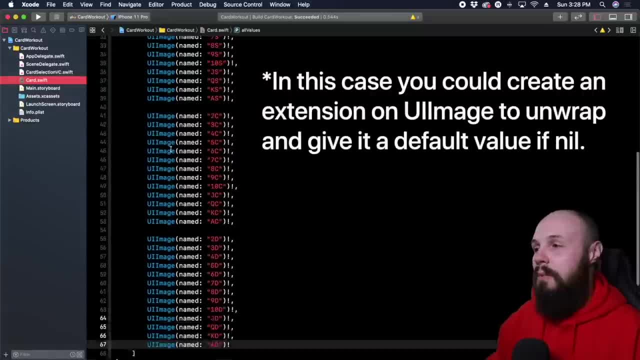 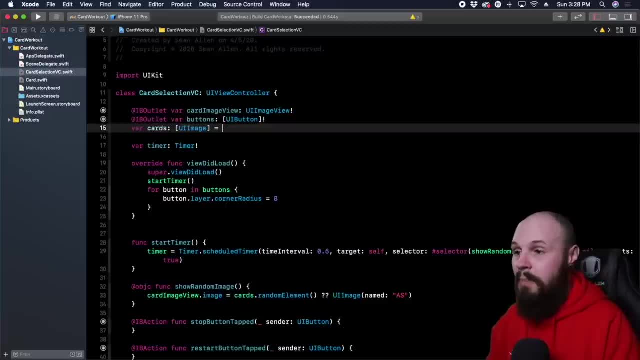 an optional. imagine if we had to unwrap. you know all 52 of these, right? so again, everything is situational. so anyway, back to card selection. uh, what I can do here in our cards array, instead of having an empty array, I can do card dot, uh, all values. 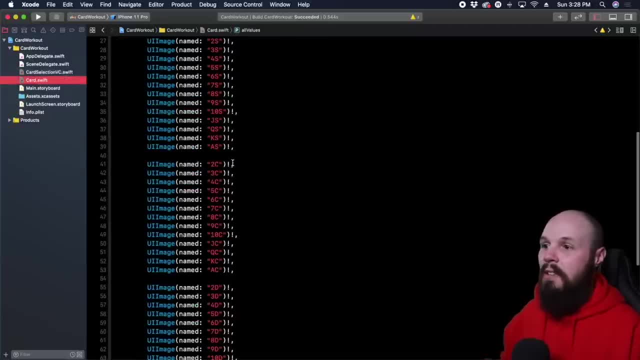 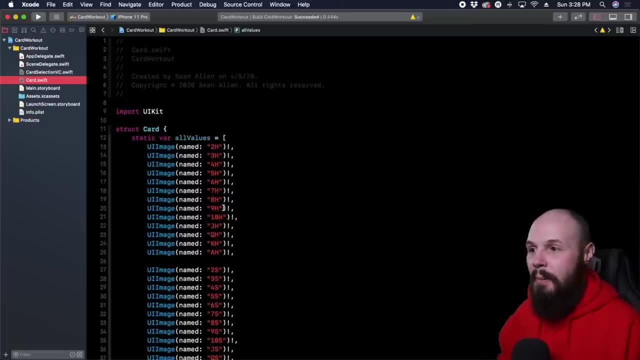 and the reason I named it all values is because if you wanted to expand on this, like technically, you could create an array of, like, just the hearts or just the spades, maybe just the face cards. right, if you were making a specific game, you know, then you could do card dot. 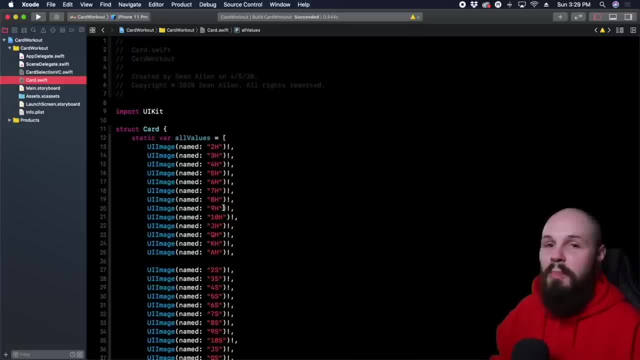 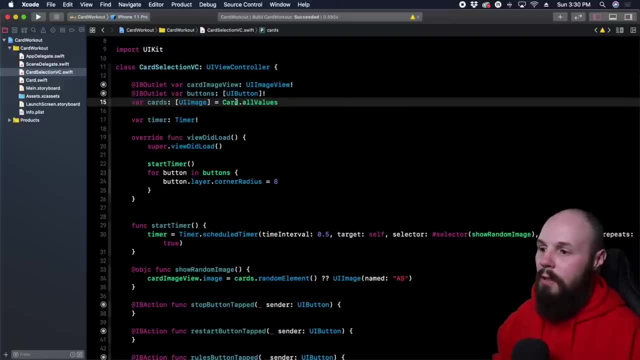 face cards: card dot hearts. right, you could really, uh, you know, subsection this uh off, so I did card dot all values. now our cards array has all those values that we just created. so, scrolling down to our random image now, when the timer fires off every half second, 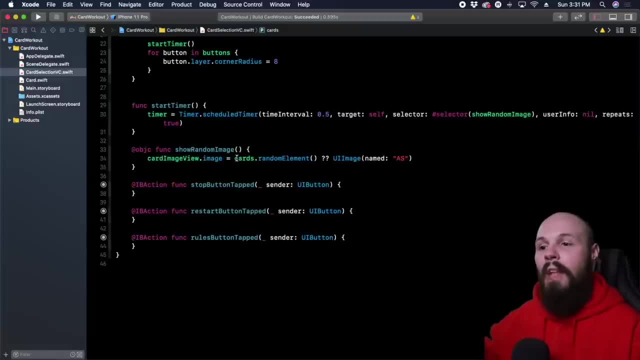 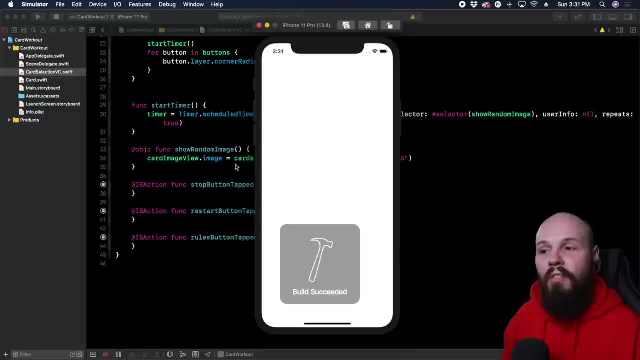 our card image view. dot image is going to be a random element from that array um. and if that array is empty, or if you get nil, it's going to default to the ace of spades. so now, when we run it, our card should change every half second. right, there you go. 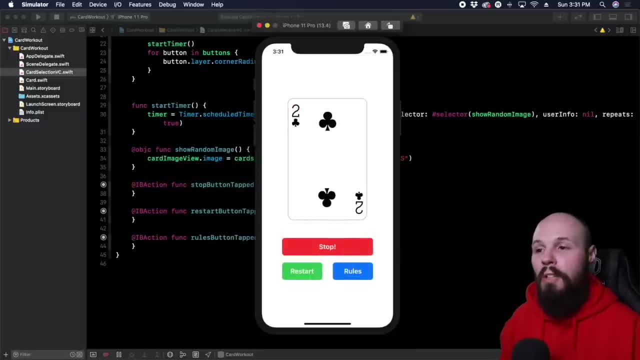 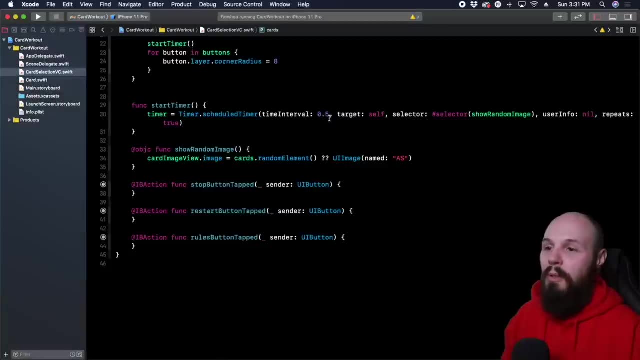 half second is changing and it's pulling out a random element from our cards array. now, half second is a little slow, right? like you can like, stop, you can like pick what card you want. so let's speed this up a little bit. let's do 0.1. 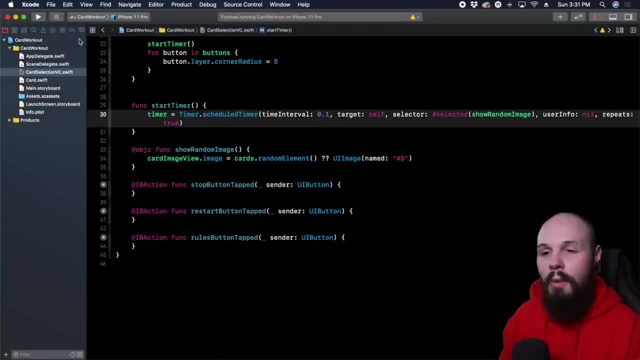 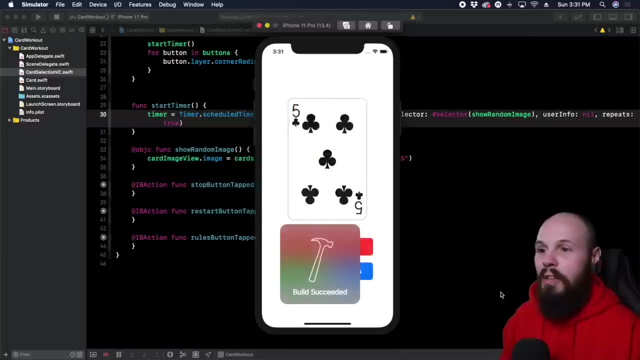 uh, and you can. you can tweak this on your own, dial it into whatever timing you like, but so this is every tenth of a second it's going to change. so now, when we run it now, you can see going really, really fast, like now, i don't know what's coming, i just 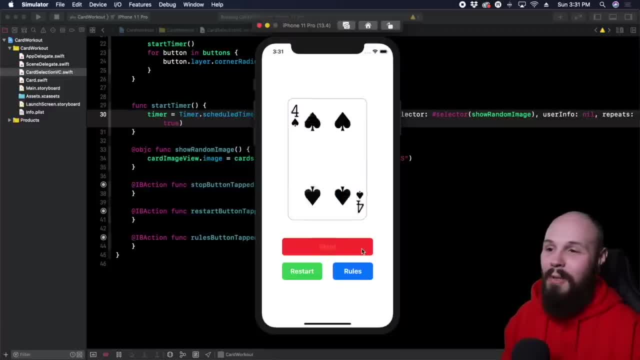 have to hit stop randomly. well, we haven't implemented that yet, so we're just, we're just firing off forever. so let's stop the uh the simulator and implement the stop and restart buttons. so stop this. so the way to stop a timer is actually relatively simple. it's one line, you do timer. 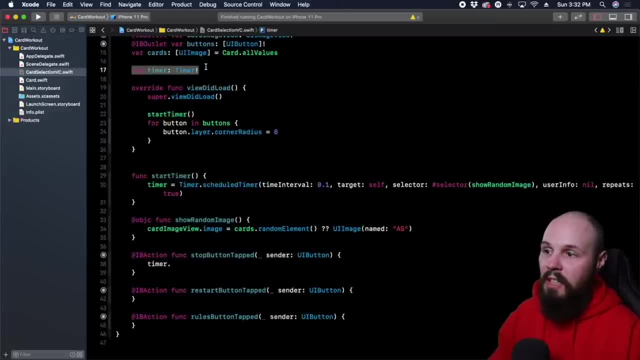 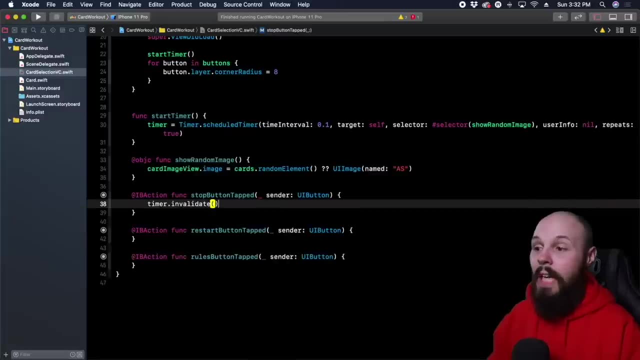 which what you know, this is the, the timer variable that we have up here on line 17, that we created and assigned a value here so we have access that timer. say timer dot: uh, invalidate, that's what stops the timer. so when i hit the stop button now, it's going to do that. 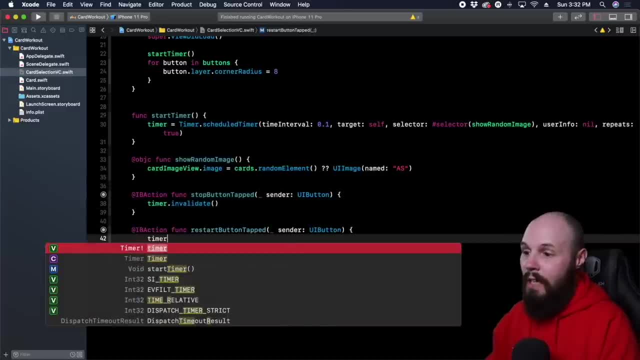 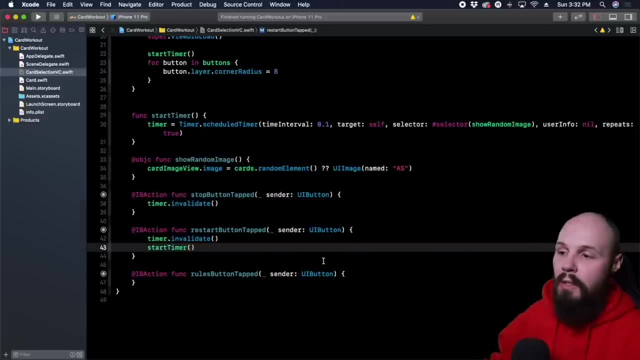 and now, when i restart it, i want to do timer dot, invalidate, wait. we want to stop the timer and then restart. that's what happens here. so start timer. so this way, whenever the restart button is, we're invalidating a timer, just in case it's already running, and starting a new. 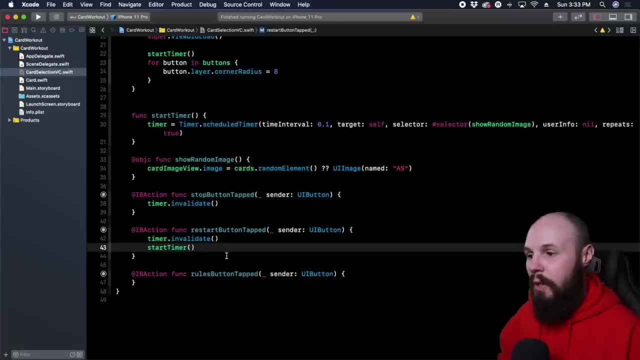 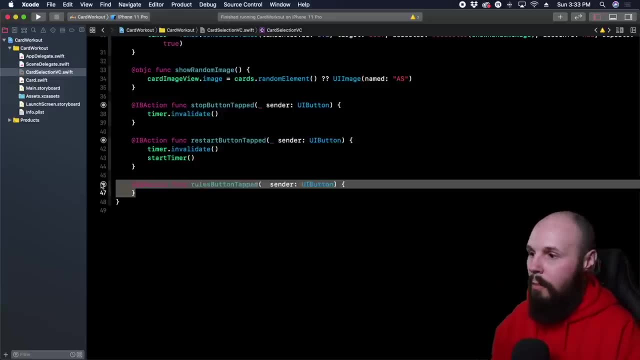 one, or if it's stopped, you know the timer invalidate doesn't fire off and we start the timer here. so rules button tapped, uh, we actually don't need that right, remember? we set that up uh before to where the button just goes in our storyboard. the button just shows it automatically. 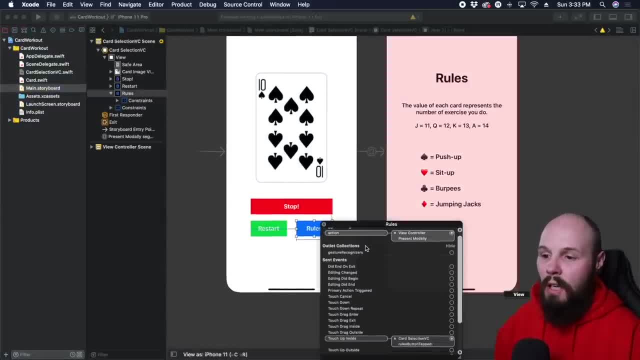 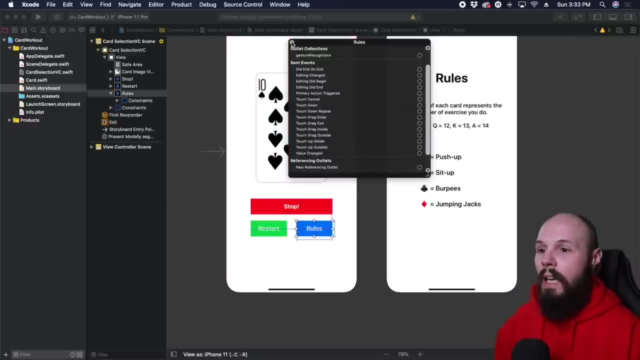 so i deleted that code. let's make sure we delete the action here. um, i think i might have already done it. nope, there's a touch up inside action here, right rules button tapped. gotta make sure you delete that. when you delete that code, uh and again, uh, we don't need that. 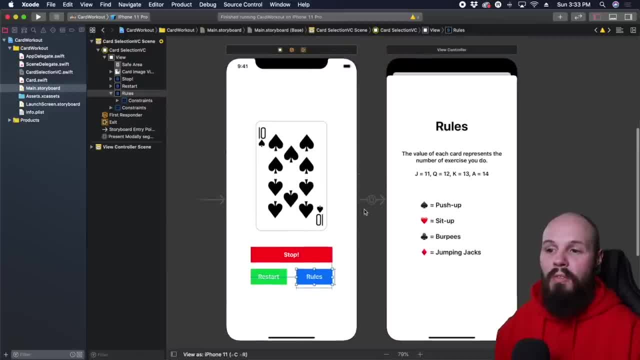 we don't need that code when the button is tapped because we based it off this segue. if remember, we just dragged from the rules right to that and did present modally in the previous video. so that is why we don't need that code anymore. so back to the card selection vc. 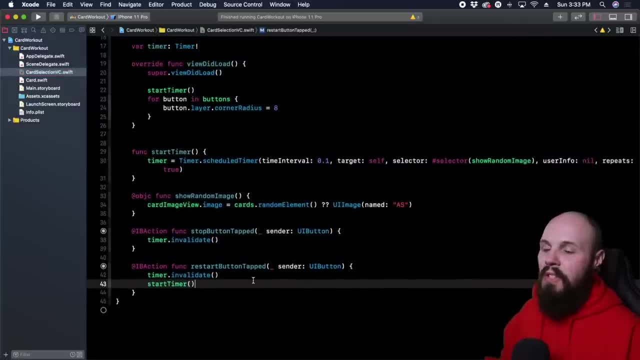 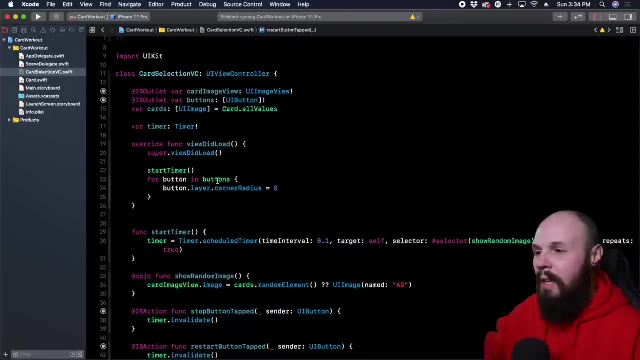 uh, we should be good to go. but before i run this and finish up the video, one quick note about timer. and again, timers can be more of an advanced topic. i just wanted to use them because it's a cool part of the app. but uh, so the timer. 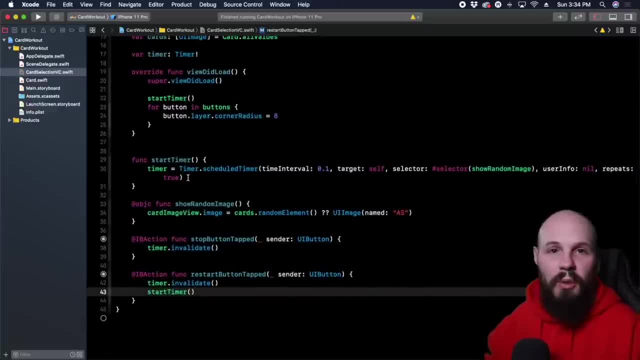 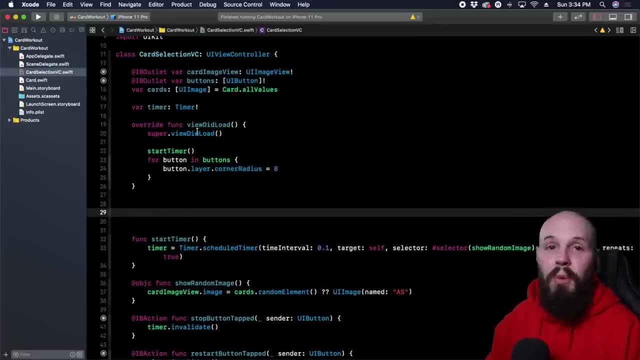 is always going to be running once you start it. so when you leave this screen, if you had multiple screens, you always want to make sure your timer is invalidated. so, uh, this is part of the view lifecycle method, just like view to load is what you started with. 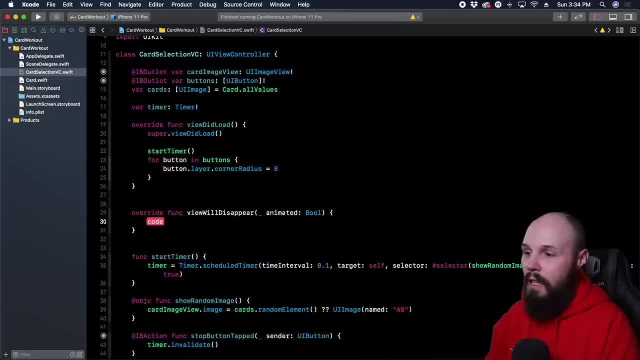 you can do: uh, view will disappear, and so call super dot, view will disappear. you always want to call the super when you're overriding. well, not always, but 99.8 percent of the time. that's the thing with programming. there's almost no absolutes, there's always like. 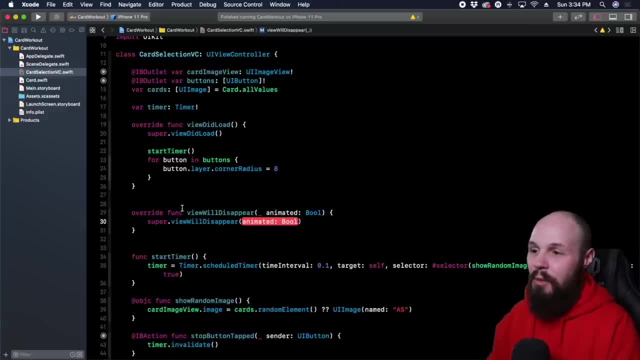 some exception, but the vast vast majority of the time. you always want to call the super and remember what that does is if you're overriding a function on the child. uh, remember the subclass. i should say you want to get all the functionality of the super class or the parent class and then add your own functionality. 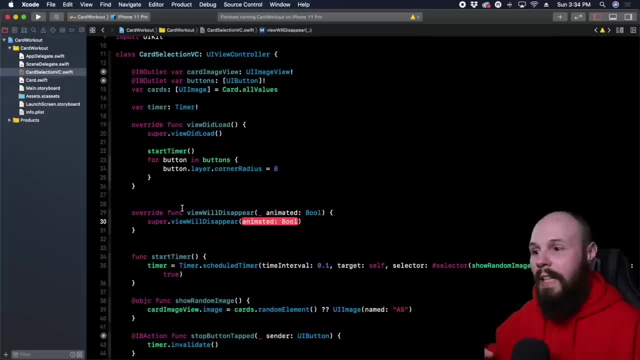 if you don't call super, view will disappear. you're not going to get all the built-in function of the view controller that apple has built for you. so that's why you want to be calling the super. when you override a function, uh, and then pass in the animated that is. 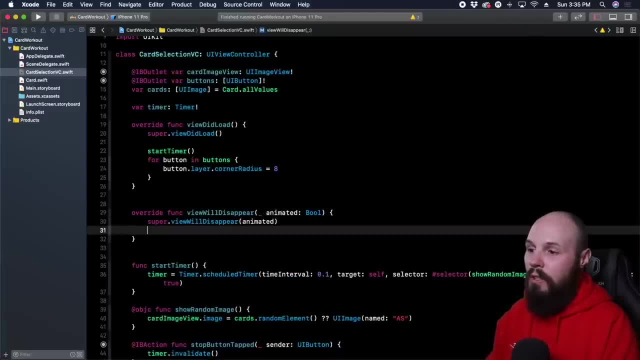 right here, we're just passing that through, so here in view will disappear. i also want to call timer dot invalidate. so there you go, and real quick at a high level. there are other uh view lifecycle methods, uh again, so view will disappear. it kind of makes sense. this is what happens, right. 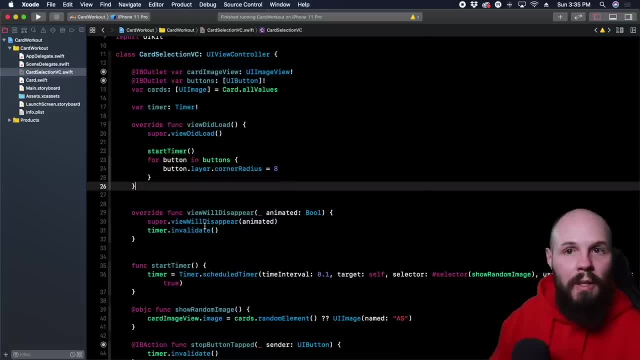 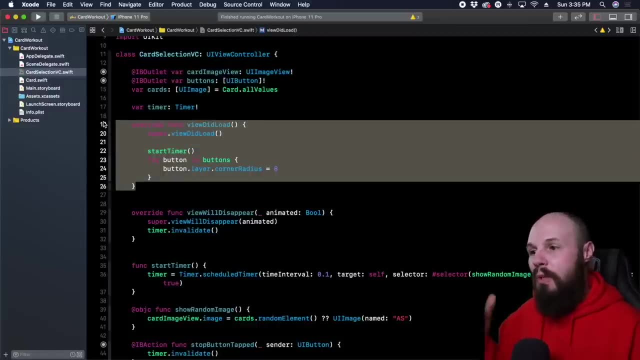 before the view disappears, there's other ones like view will appear. that happen right before the view appears on screen. as you can see, view did load. this is what happens when the view controller is like loaded into memory. um, so there's various view lifecycle methods. i'm going to link to a video in my youtube. 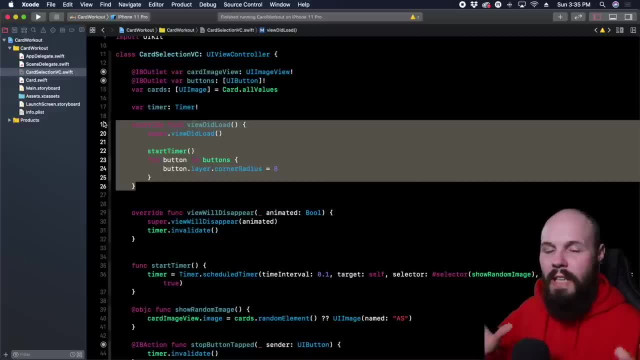 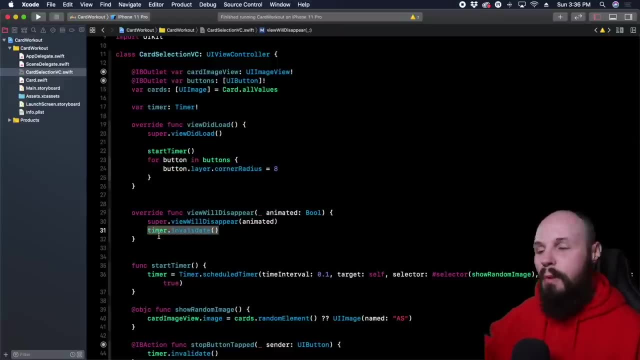 about that rather than diving in fully here, because i explain it in depth in the video. um, so we want to make sure our timer is always invalidated? uh, because, again, if we don't invalidate that, it's always going to be running in the background and that's just bad memory. uh, usage here. 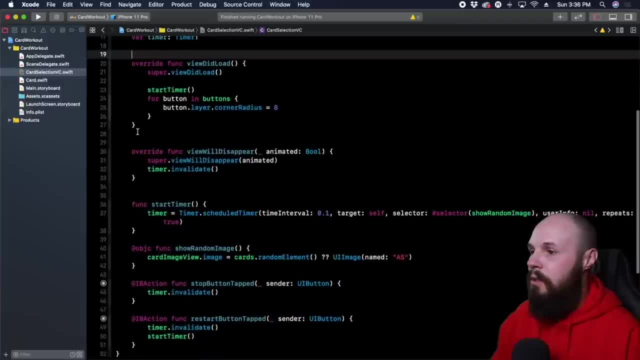 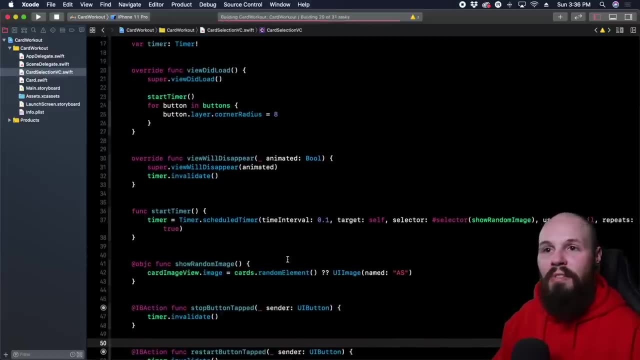 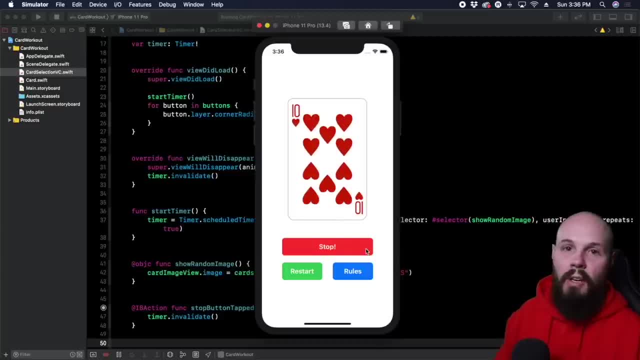 okay, so timer's running, timer's running. cool, stop, all right, ten of hearts. so i would have to do ten sit-ups? i believe not gonna do that. uh, restart, there we go, we're back up again. okay, cool, stop done and restart. and then now, when we hit restart, 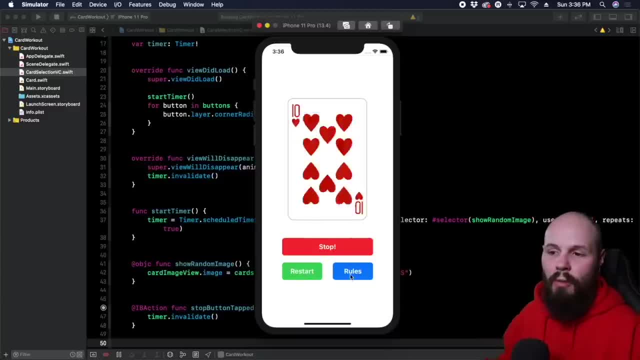 still, it still keeps firing off. um, so we're good to go. and if we ever wanted to see the rules, okay, cool, those are the rules of our game. swipe down, still going on. uh, stop seven hearts, gotta do seven sit-ups. so again, if you want to use this app to practice anything, 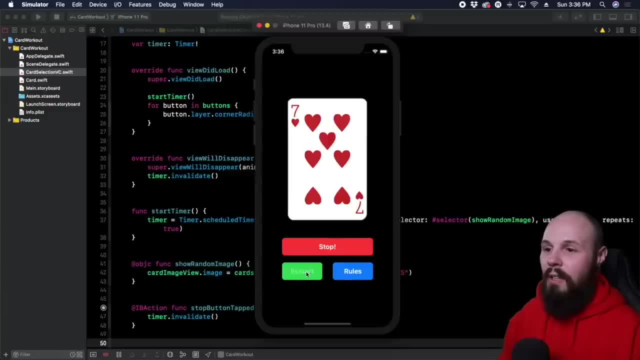 and then okay, as always, i like doing this command shift a uh restart. we're still working, even in dark mode. gotta love it stop. all right, eight jumping jacks, i believe. yeah, rules, diamonds are jumping jacks. there you go. so, yeah, use this app, have fun with a workout or anything else you want. 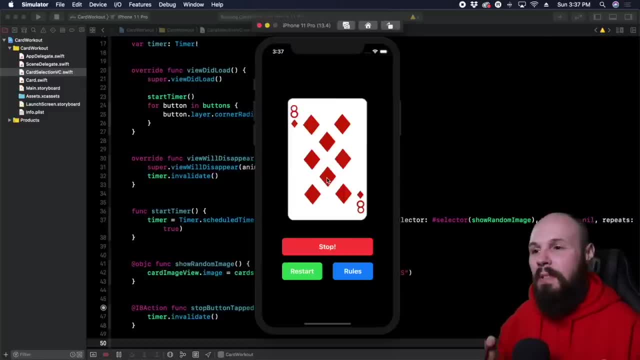 to practice. um, but that wraps up the storyboard aspect of the app. uh, again, we are going to rebuild this, but all programmatically, and do a little bit more um, refactoring, like i said, with the custom ui button that we're going to create. so, again, a lot of this was. 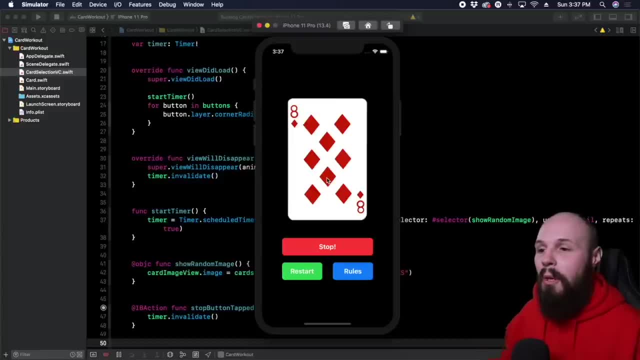 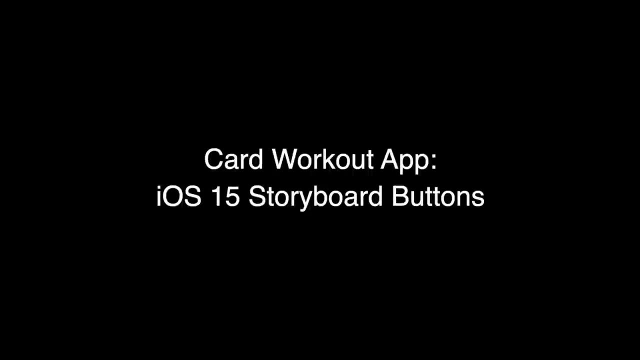 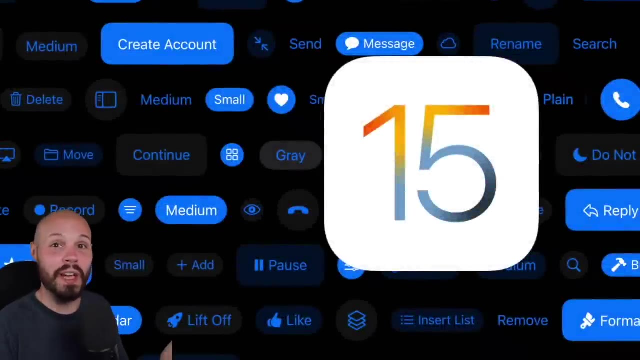 hopefully review again, just repetition, doing drills, you know, building up on our skills. but again, next video, all new stuff. hope you're ready, let's go. ios 15 has introduced new buttons for us. now, before you get all worried, this isn't like a complete revamp of a button. 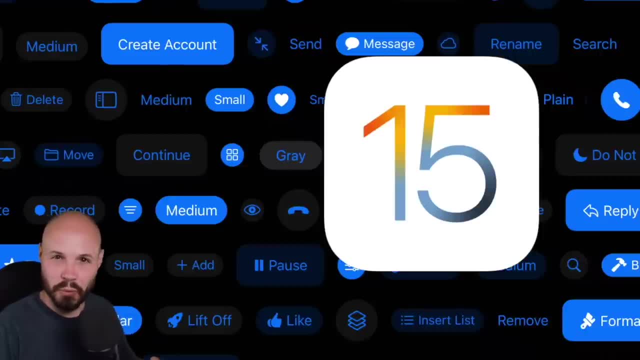 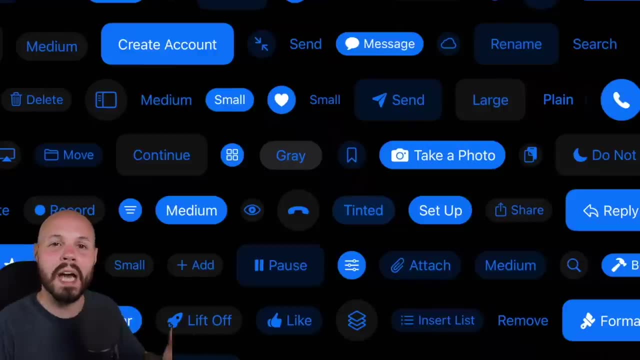 and you gotta learn everything new. to put it simply in the real big picture, these new button configurations are essentially a way to give us apple style buttons out of the box, so we don't have to recreate them. what do i mean by apple style buttons? we'll take a look on. 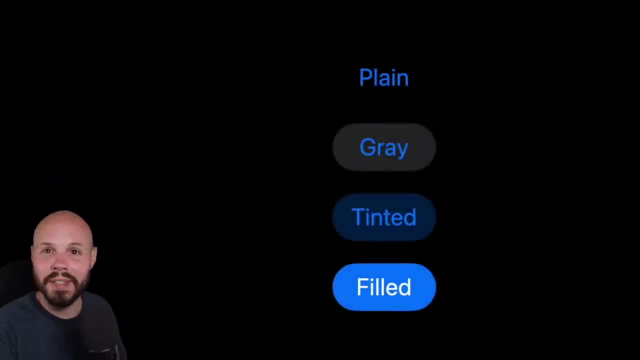 the screen. we have a plain style, gray style, tinted and filled right. you've seen these buttons in ios. so essentially what these button configurations do, or make it easy to get these styles right, if you still want your own crazy custom button, you got to do that on your own. 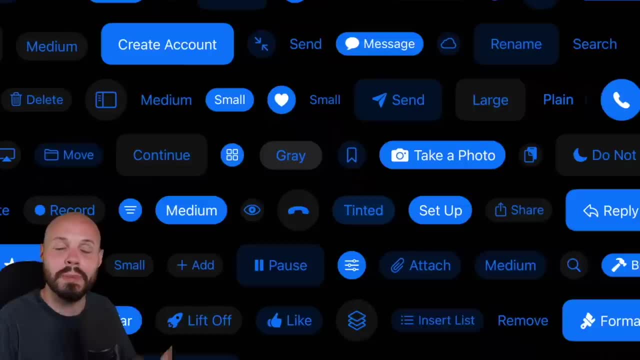 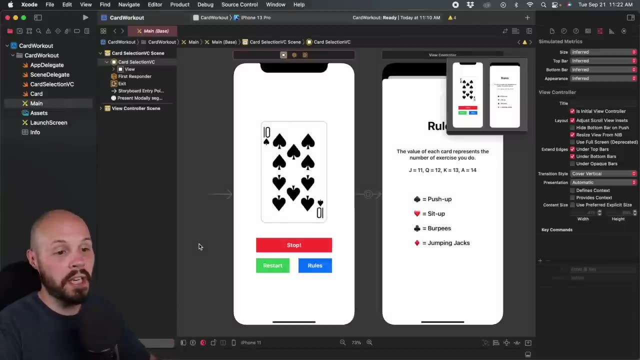 but if you want your app to feel like it belongs in the apple ecosystem and use these styles, apple now gives them to you kind of for free, out of the box. in this video we're going to convert the buttons you see here in our card app. right the stop. 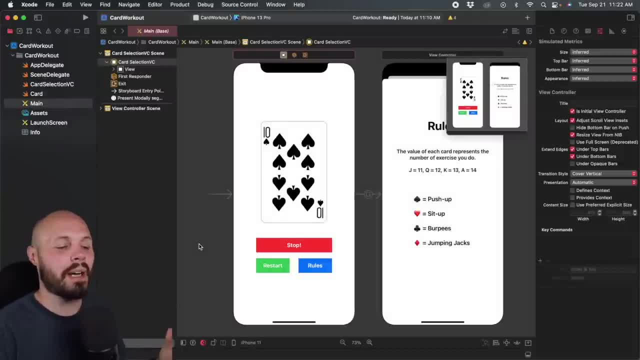 button, restart button, rules button, and we're going to play around with these new styles using these buttons. now there's a new wwdc 2021 video that goes into these buttons in depth, because, again, we're going to keep it pretty surface level, pretty introductory, because this is 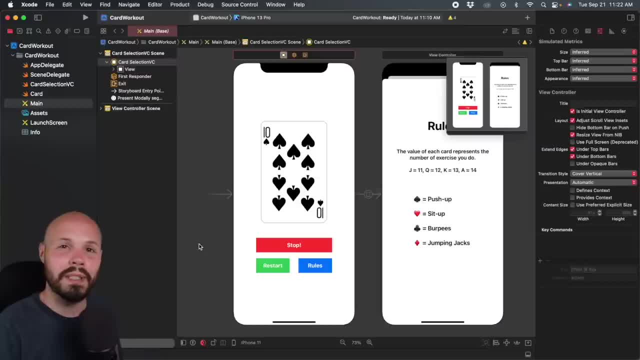 the you know fundamentals, course, but if you want to dive deeper, definitely check out that wwdc video, and there's another video i'll attach there- all about the new stuff in interface builder, which again shows you how to use these buttons as well. okay, so, as you can see, i got my main storyboard. 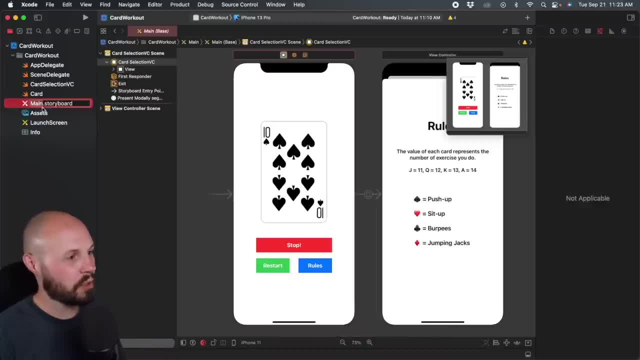 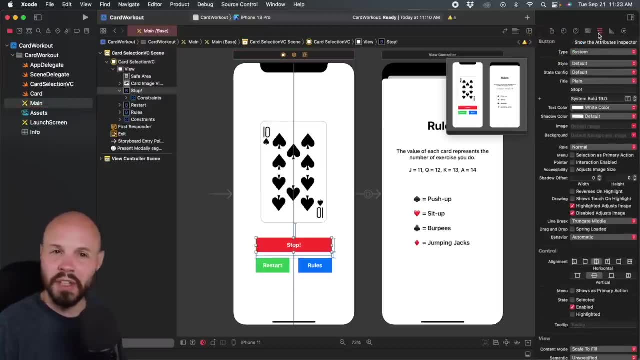 selected. you can see the new icons in xcode 13. i think those look pretty cool. click on the stop button and then over here on the right you'll see the attributes inspector, which i think these might get some new icons again. i didn't include that in a whole. 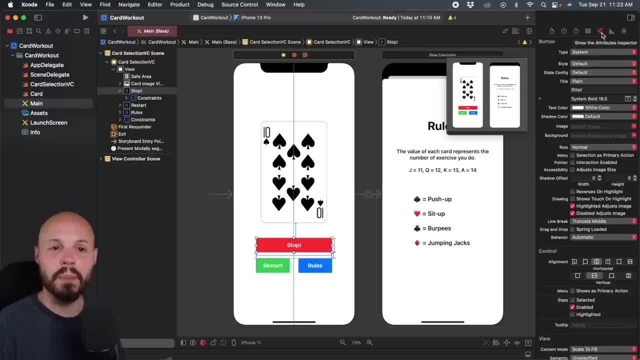 separate new video, but some of these icons have changed, but they're still in the same spot. but we want the attributes inspector and, you see, the main thing here is style right, so right now it's default. so these are the styles i mentioned, right, plain gray, tinted filled. so let's start with 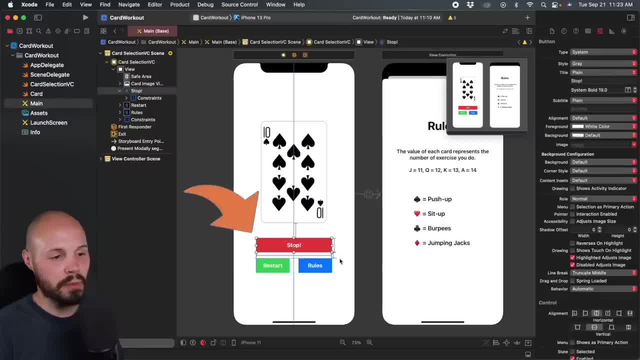 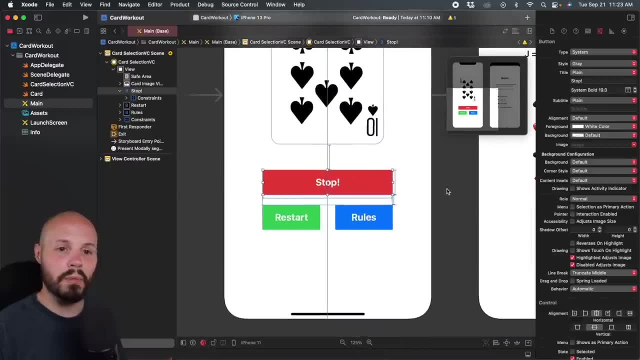 gray. so if i click on gray, you'll notice nothing really changed with my button down here. here i'm going to zoom in on my buttons like even more, so we can like make them real big and see them now. the reason being is because we still have our background color of system. 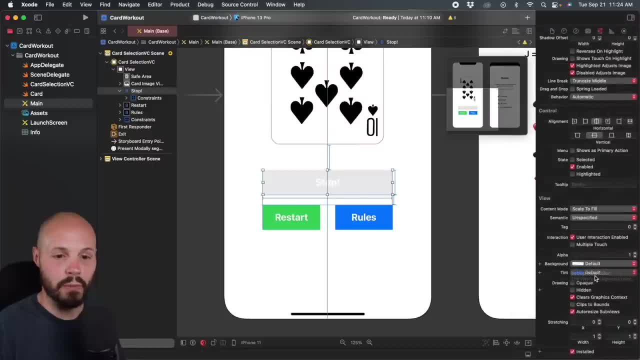 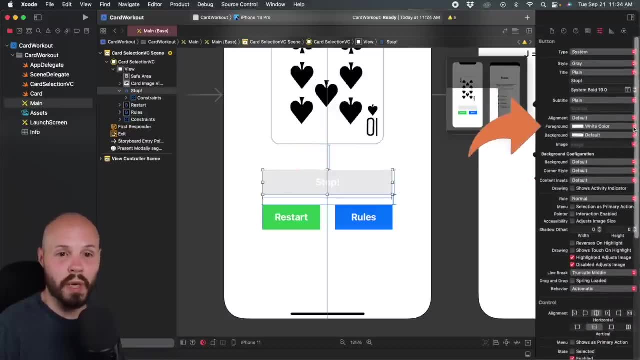 red. so if we get this to default, get that out of there, we'll no longer see that. so now we have gray, but you'll see our text is still white. see this foreground. that's a new attribute. it's white color, so we'll change this again. 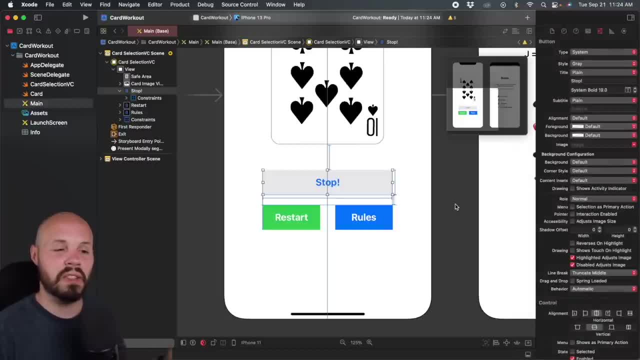 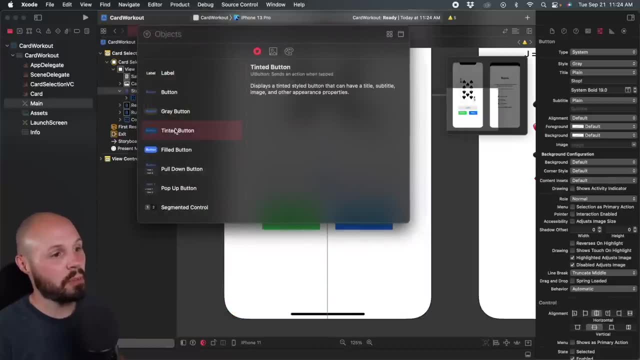 back to default. now. this is us adjusting our existing button. one thing i want to show you again: if you do command shift l to get your object library out here, right, you see we have gray button, tinted button, filled button. you can drop this in. if you were starting from scratch. 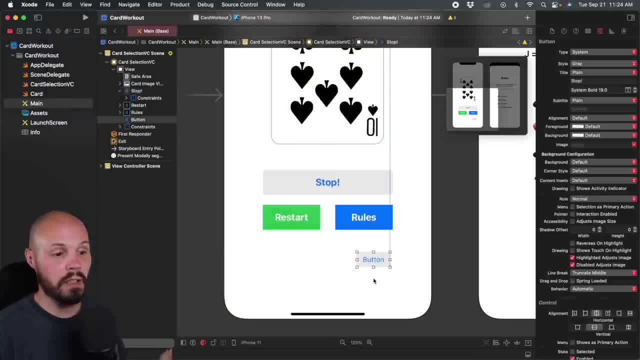 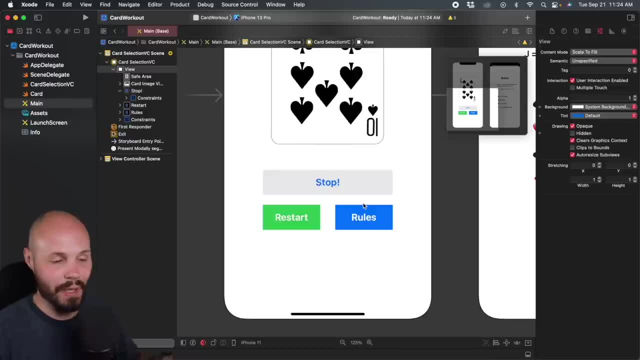 again. so let's say, you did want a gray button and we're starting from scratch. you just drop that in and you get that look right. we only had to, like, go back and change that stuff because we, you know, had existing styles, we had an existing button. just want to. 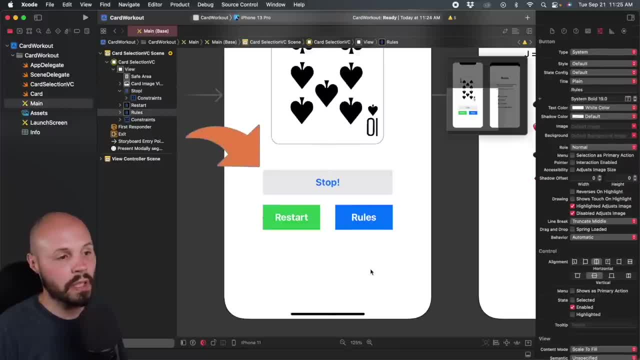 be clear on that. so back to our stop button. i'll click off of it. you'll notice we get a little bit of a corner radius and that's part of the default style. so click on this button so you see that's gray. and now that we have, like, all the default, 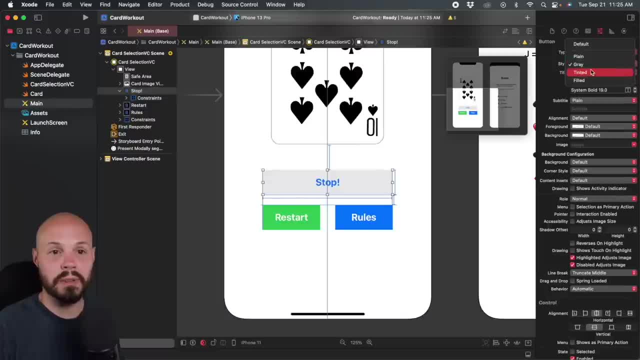 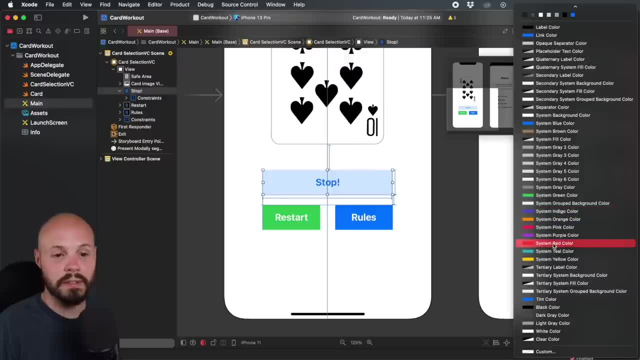 set. we can kind of change this around a little bit. so if i want to go to style tinted, right, so now that's the tinted blue, but now i can change the background color. let's say we want like a red tinted, so system color red. 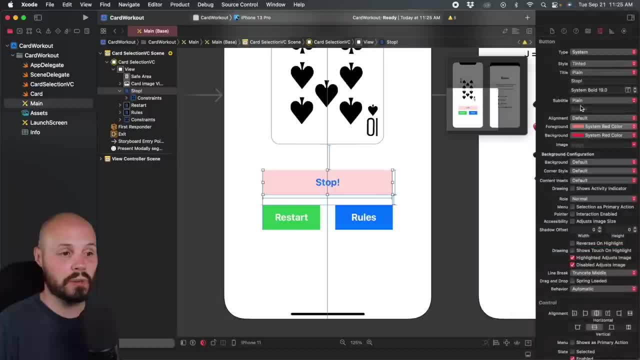 and then the foreground color is also system color red. so again, the foreground color will change your text. the background color will change the background, but we made them the same color because this is the tinted style. it gives us that. you know, light red background and dark foreground. now this is. 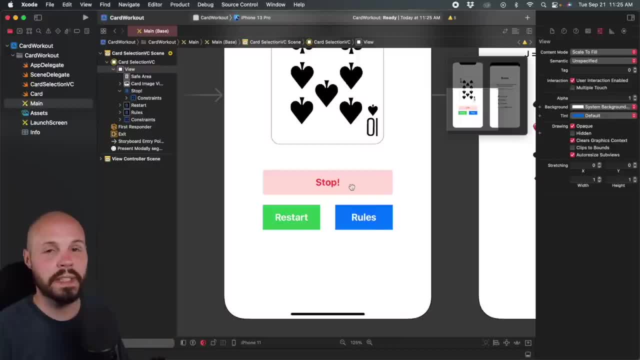 good for contrast ratio because if you use the same color you're pretty much guaranteed a good contrast ratio for, like, visibility purposes, or sometimes, like you know, white letters on a yellow button- you know you can really see that, so this ensures good contrast. or if you just like that look and then 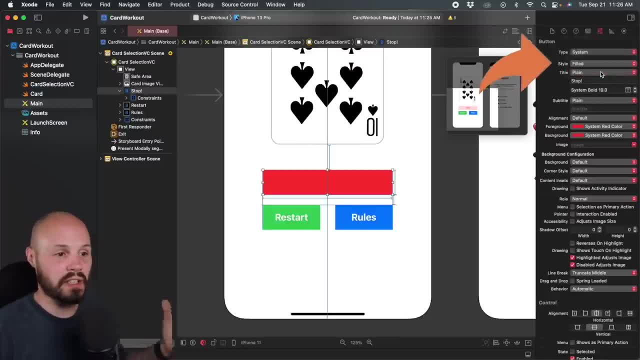 again back here. uh, we'll go to filled. this is kind of the style we did have, except, you see, our foreground color is still red. now we want to make that foreground color. we can make it whatever you want, but we're going to go with white to give us that back. 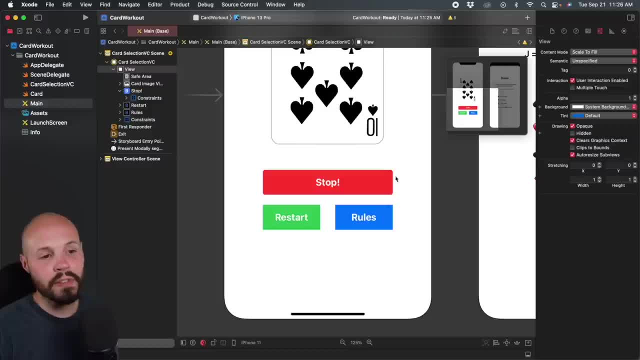 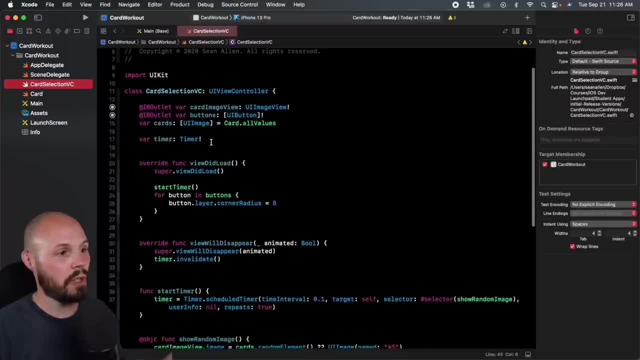 so that is the general shape of it, but you'll notice right our we have a little bit of a corner radius, whereas before, on our rules and restart, we had to set that in code. i'll go to the code to see if you remember that right, see where we have our out. uh. 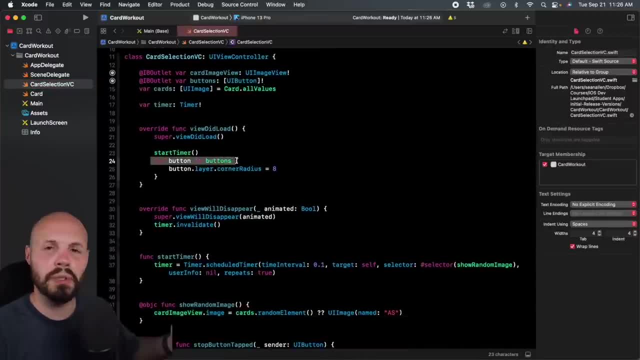 yeah, outlet array of buttons here and it we do our for loop. hopefully you just kind of did this a little bit ago, so this is fresh in your mind- where we iterate through that, all those buttons, and set our corner radius to eight. we do that in code but it doesn't show up on. 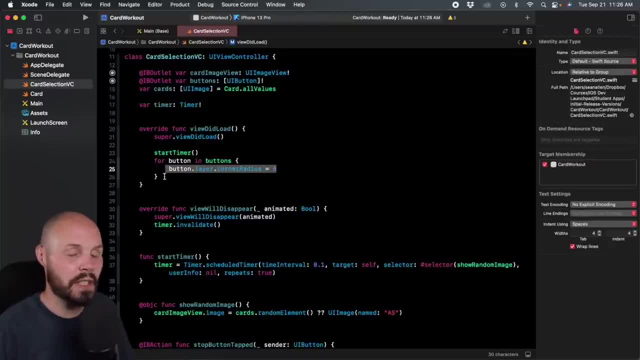 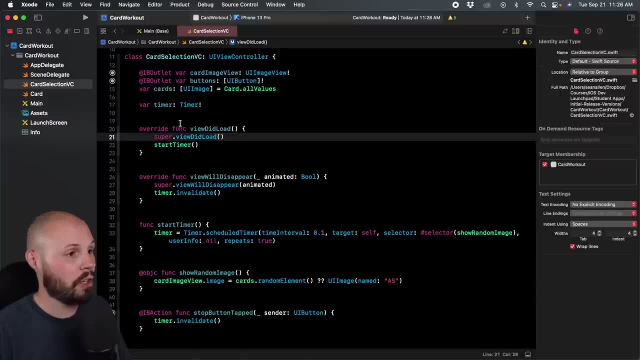 our storyboard. well, that's. another benefit of these new styles is you get the built in corner radius. we're going to play with that in a little bit, but first i want to delete this code. we no longer need that code, so therefore i no longer need this uh outlet. 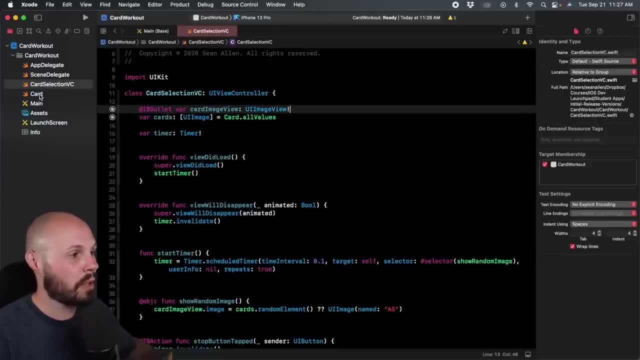 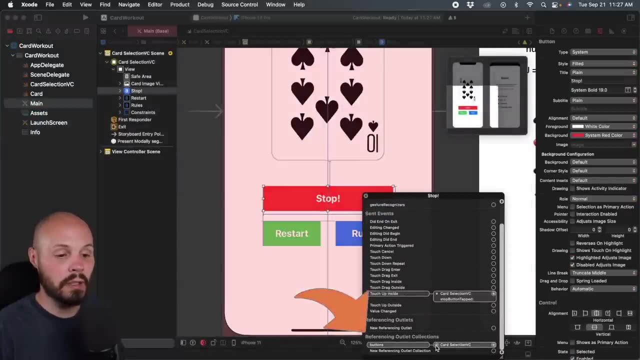 collection of buttons so we can get rid of that. and then remember, go back to our storyboard, make sure you delete that, delete these outlets. so right click, you see, uh, this referencing outlet down at the bottom, uh, in the array of buttons. get rid of that. we'll do that for all. 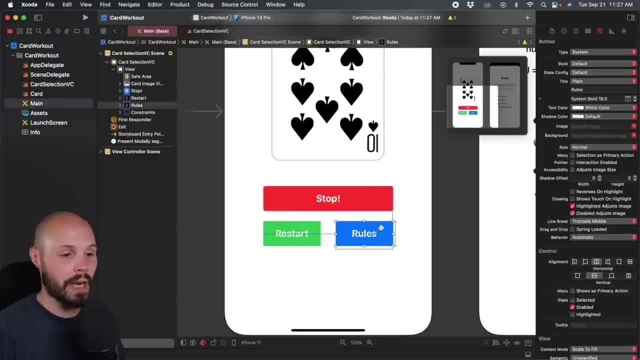 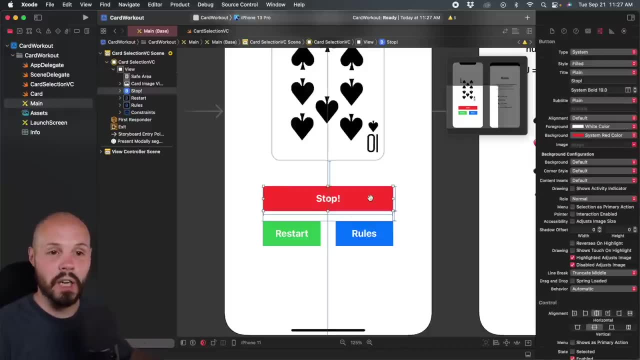 of these because- remember the thing with outlets- you got to make sure to go back and delete them if you no longer are using them. so cool that is done. but now you see, we get these corner radius for free. let's talk about this corner radius a little bit. 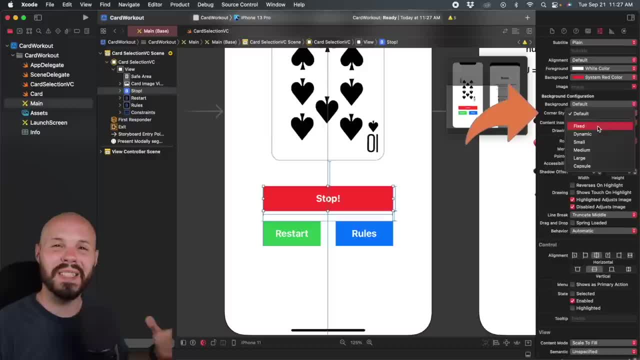 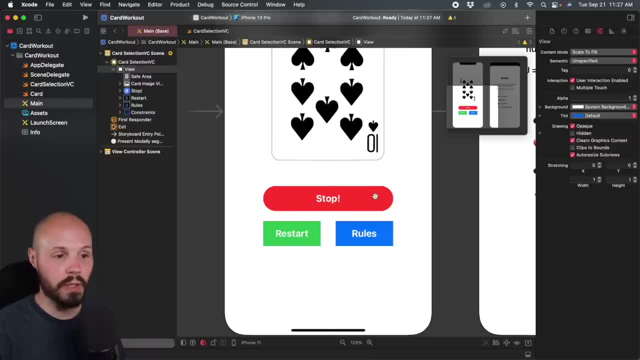 here you can see, on the right we have corner style default. uh, we don't get to set the exact number but you just kind of get. you know, small, medium, large capsule. so capsule will give us, you know, that circular look that you're probably very familiar with seeing. and then if 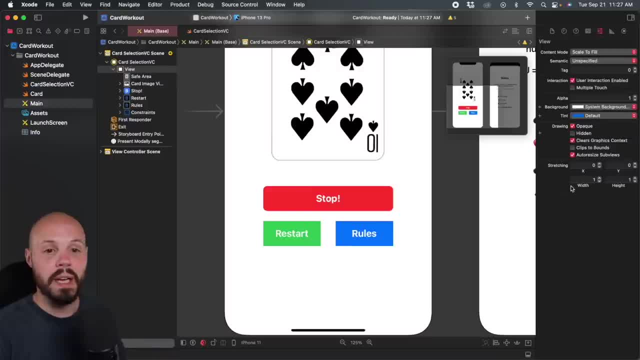 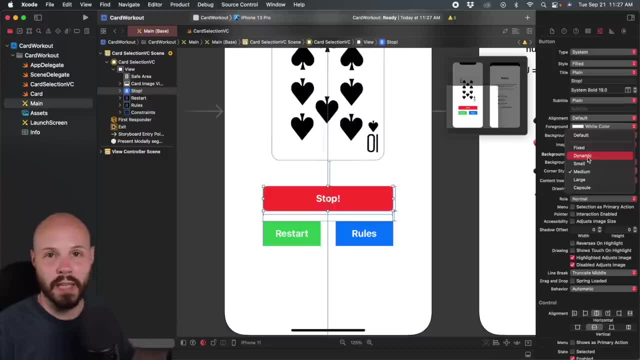 we want to do, like we'll do medium. that'll give us a medium corner radius and then if you notice the dynamic one, uh that you might have seen here- corner style dynamic- that will change with, uh, dynamic type, right, so as the button text gets smaller or bigger, uh, that'll be dynamic. 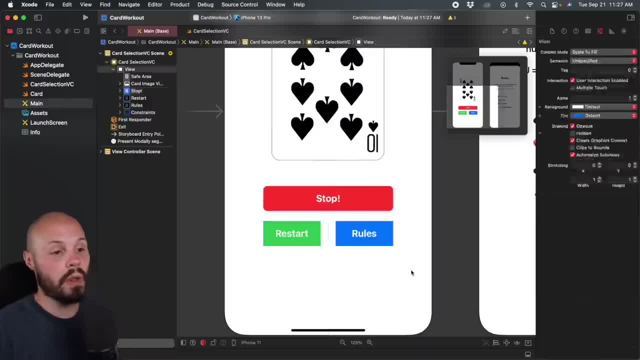 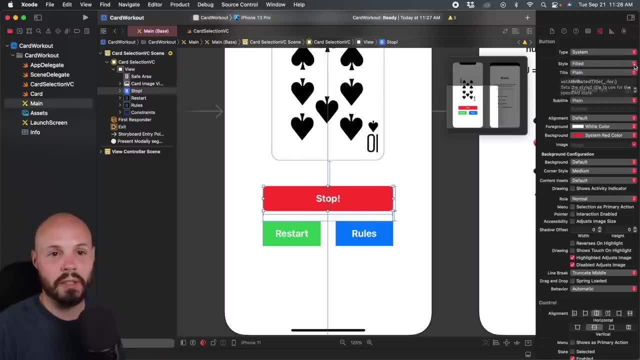 but we're just going to go with medium or pick whichever one you want here. so that is basically the button style. so we went off that with stop you know what. let's change this to tinted. uh, just, i like this look right. so sorry, style not filled. uh, we'll do tinted. 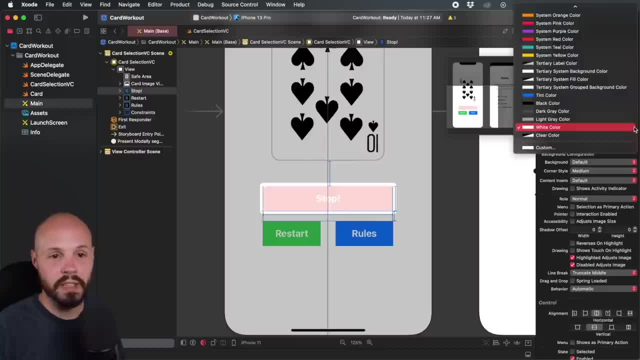 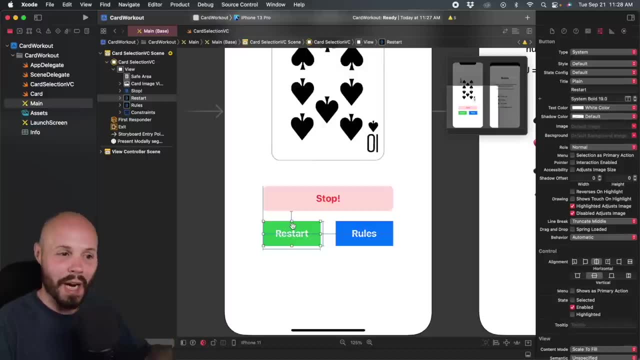 but again, we don't want our foreground color to be white on tinted, we want it to be, you know, system red again to get that color. so let's do the same thing with our restart. um, actually, if you want to like, pause the video and try to set up your restart and rules. 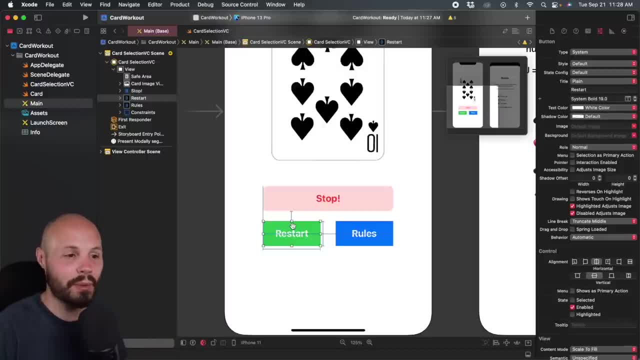 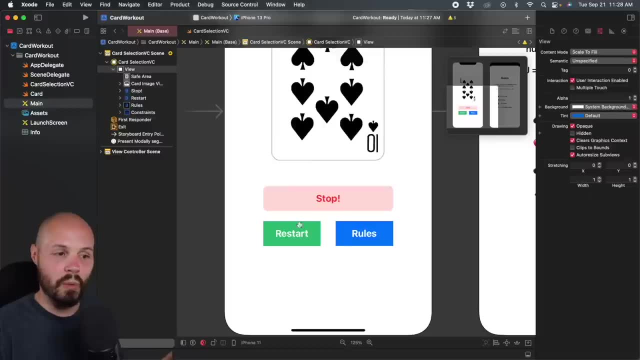 buttons accordingly. go for it. nice little challenge, but i'm going to do it right now as well. so again, on the restart button, we want to give it a style of tinted and then up. you'll notice, like i said, it didn't quite change it because on our 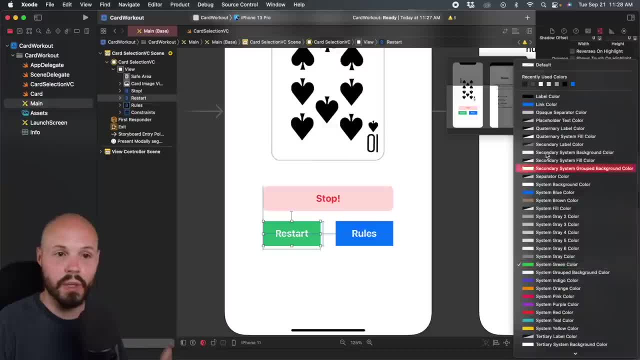 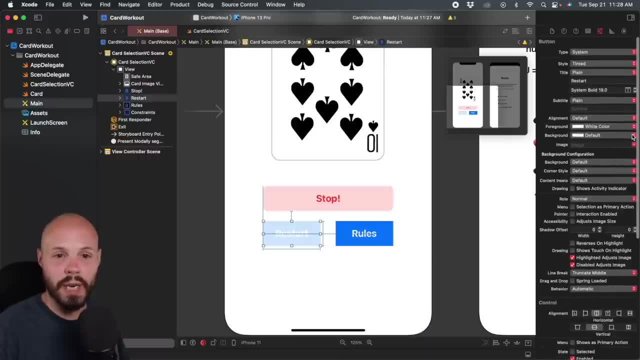 button. we still have our background set down here again, because we are using existing buttons. we got to kind of go back to the default stuff, so we'll scroll up now. we got to make our foreground color- uh well, the background- not default. we want uh system blue. and then also for the 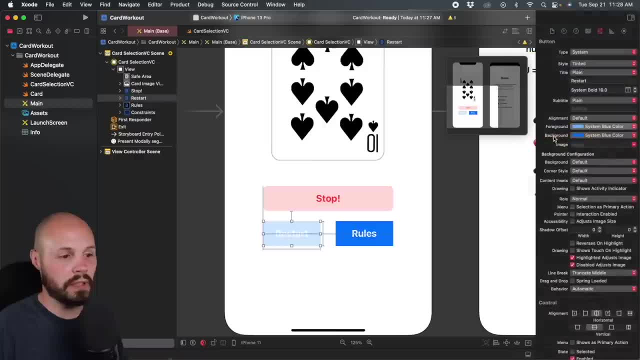 foreground. color system blue. again, when you're using the, the tinted, you want the same color for both. okay, actually this, this was green, my bad system green and system green. there we go. same thing for rules. oh, and then corner radius: we wanted medium. right corner style: medium. 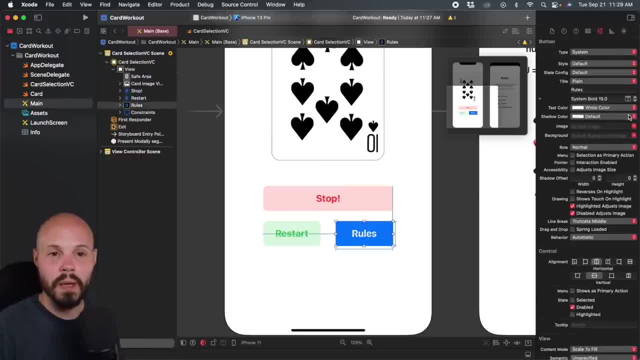 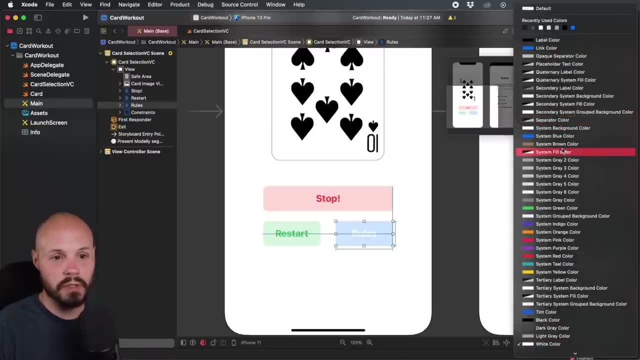 and then we're going to add images to this as well. real quick. so change our background color back to default. down here, back up here. we want style to be tinted and corner style. we want medium and then foreground, which is our text. we want to be uh system. 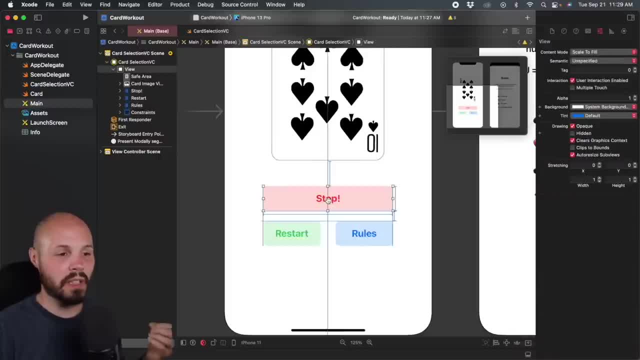 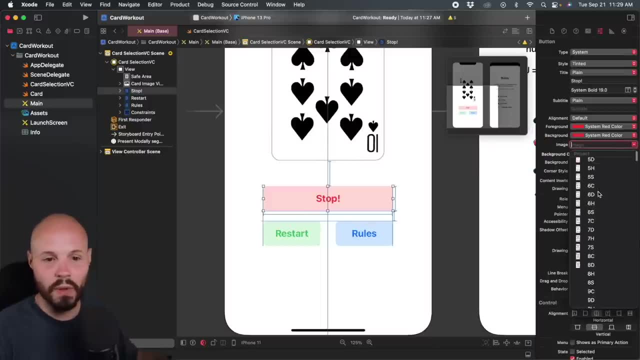 blue. so there you go. now let's talk about adding images to this, because this is a nice little free thing. we get as well. you see this image field down here. stop, uh. well, okay, these are all of our cards. we don't want that, but here we get sf symbols. 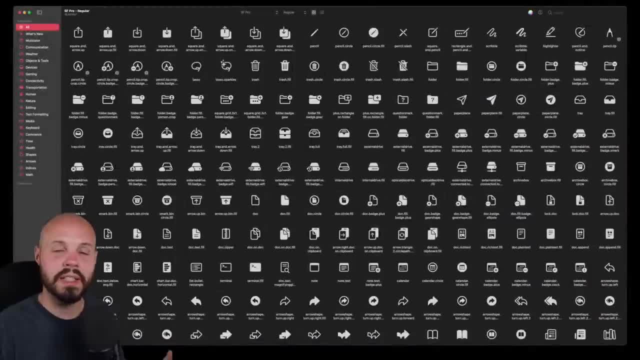 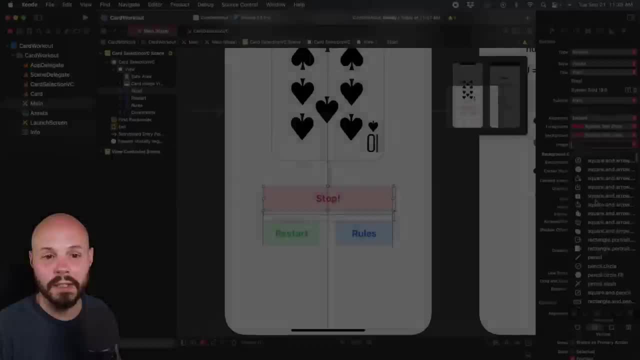 i don't think we've touched on sf symbols in this course yet, but sf symbols, as you can see, here is a separate program that allows you to pick apple icons right. they're already like pre-made here, so you can see here's a bunch of them. so what's a good stop one? i don't know if this. 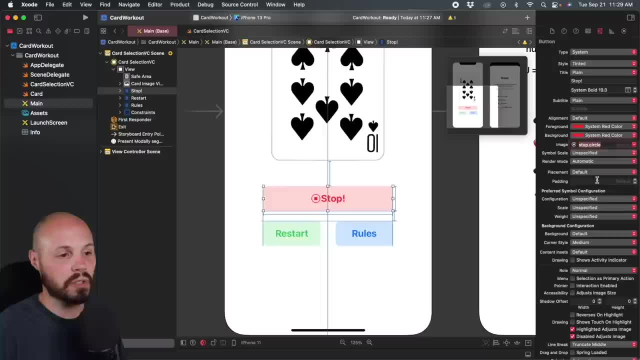 has a built-in search. i guess it kind of does so. yep, we'll do stop with a circle. there you go, and you see it's a little tight, to the words uh there. so you see you can add some padding here, right? so i'm going to add a little padding and as i'm clicking, 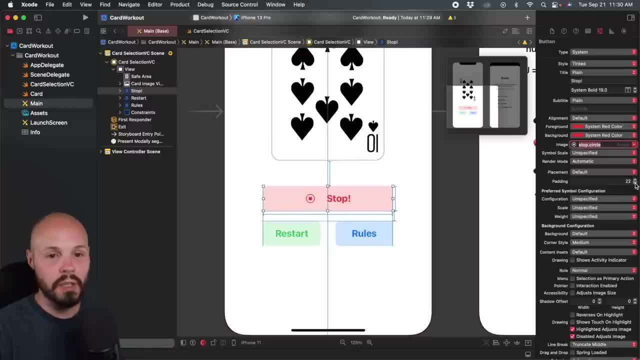 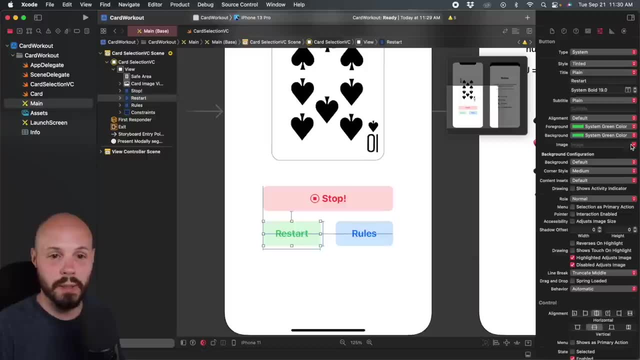 up. you can see the image. i'm going to go way far. you can see the padding on there. so put this to a number that looks reasonable. let's say that looks, that looks fine. you can do the same thing with our restart button right image. um, i'll do refresh. 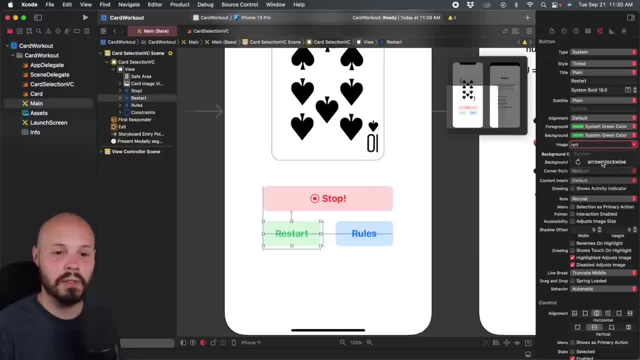 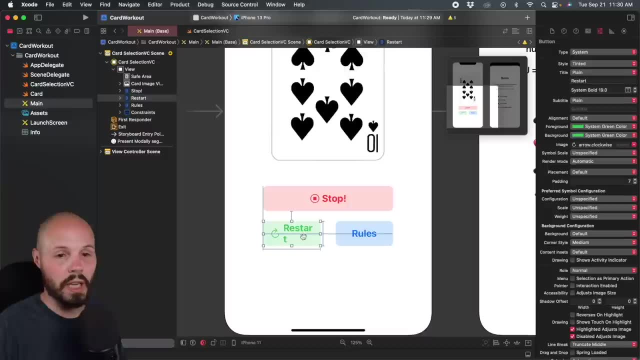 that's kind of what i have in mind. yep, arrow, clockwise, right. so there you go, use that one, and then we'll add a little padding here as well to make that look good, and then oh okay. so see, i guess i had a little too much padding. 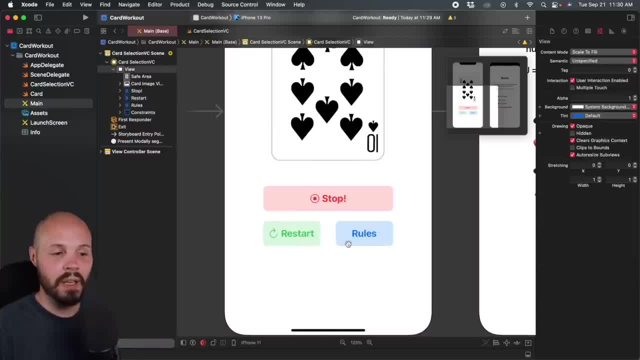 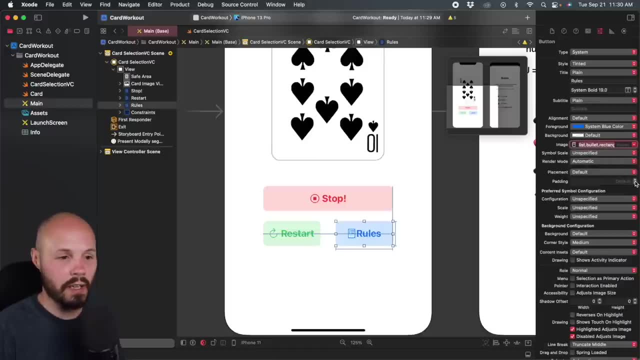 uh, you see, the restart wraps around, so be careful there. and then rules: uh, let's see here, uh, list, yeah, that that looks fine, right, list? and then we'll give that a little bit of padding as well. so, just like that, we added images to our buttons to spice that up. 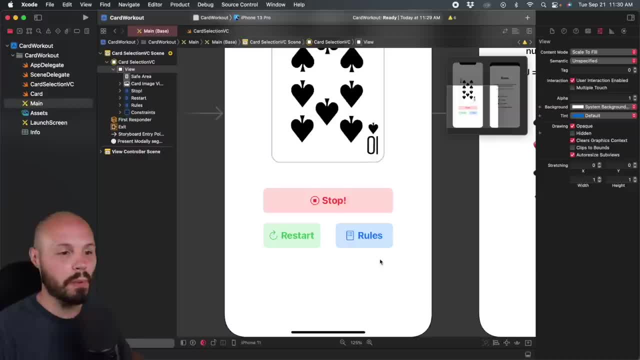 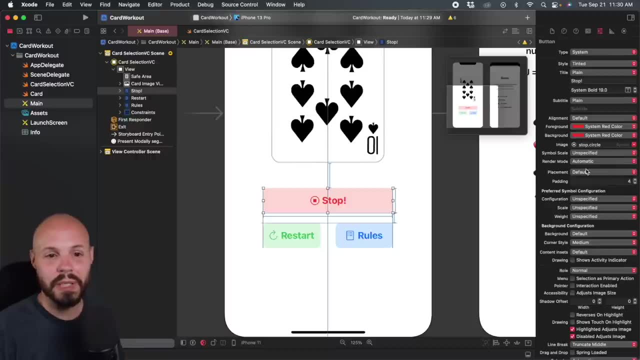 a little bit so and again, that was relatively easy. now, before we wrap up, go to the stop button. you can see all this stuff here on the right on the configurations, the way, the background corner, you can add images, placement, render modes, like there's a whole bunch of stuff that you can play around with and experiment. 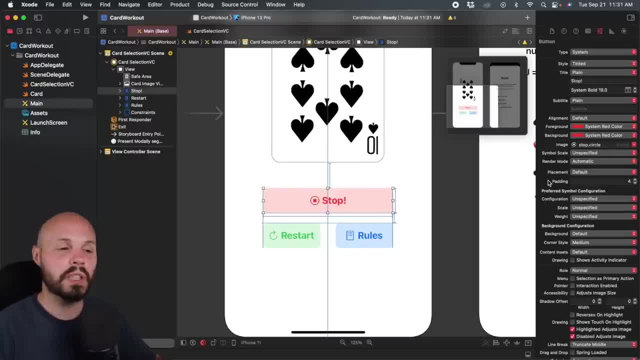 with and again. the wwdc videos that i linked to will explore this more. but again, great new button system. if you want the apple default style buttons, you get a lot of the work done for you, which is always welcome. in the next video, we're going to basically do the same thing. 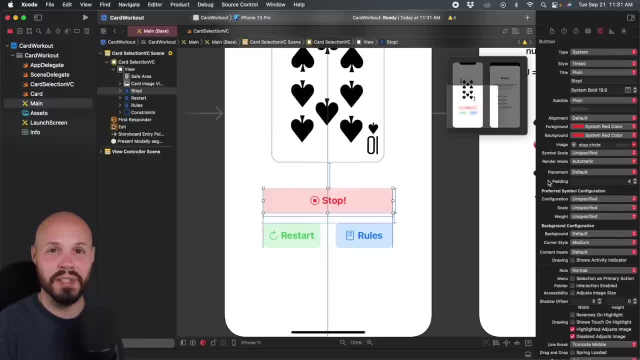 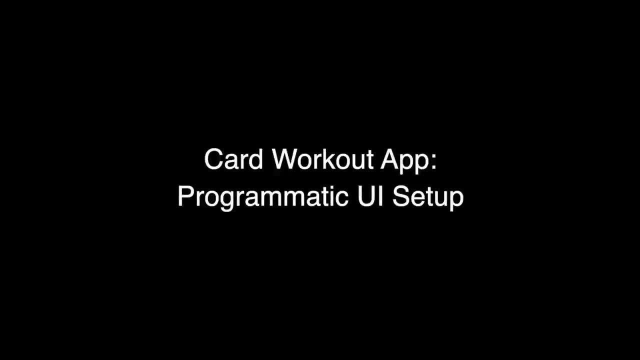 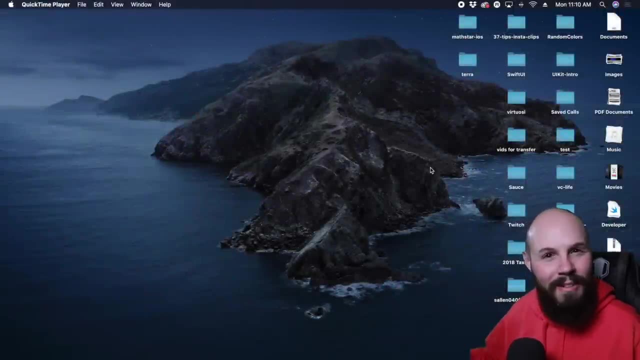 except we're going to do it in code on the code version of this app. so see you there. all right, let's begin the adventure into programmatic ui. oftentimes this is kind of daunting for beginners, so we're going to take this step by step, but again the whole purpose. 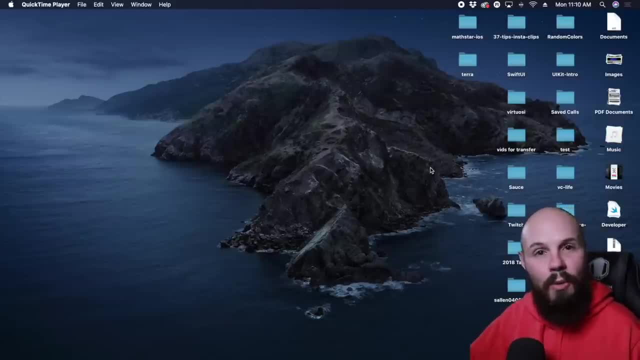 of doing this is so you can see how to build a project in storyboard and see how it's also built in programmatic ui and then start to form your own opinion, you know, in that debate. so, of course, to get started, here we go. we have to create a. 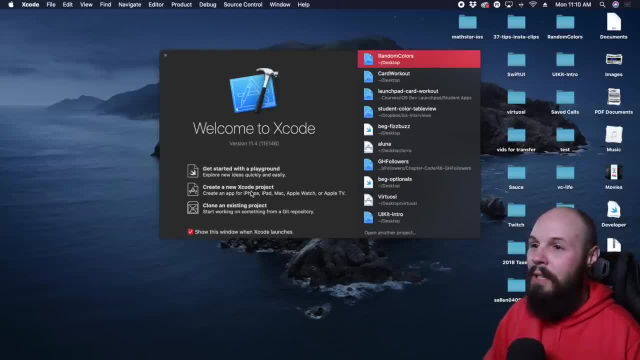 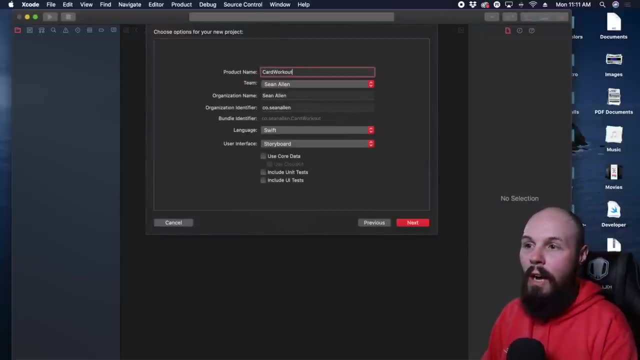 new xcode project again. hopefully we've done this a few times by now. create new project and single view application. i'm going to name this card: work out dash programmatic. i think that's spelled right. is it two t's, one t's? i don't know who cares. 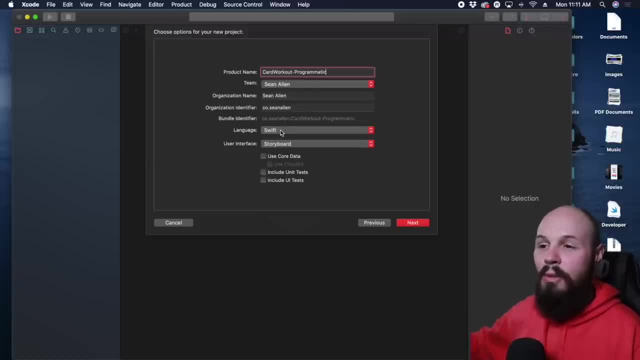 card workout programmatic again. team sean allen: whatever, whatever language. swift- now here you may be confused- interface storyboard. well, i said we're not using it, we're using storyboard, so the other option is swift ui. we're not doing swift ui, so we have to select storyboard and 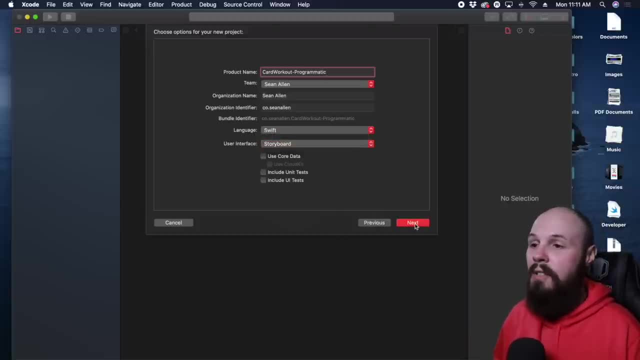 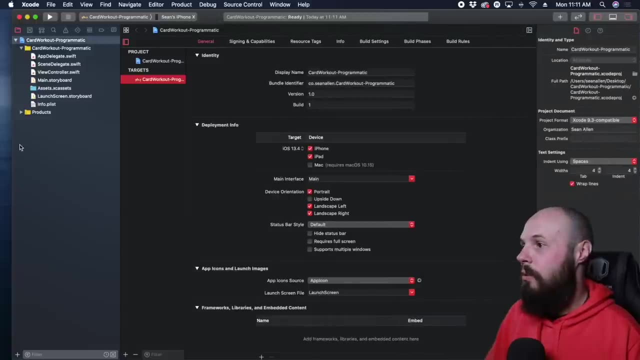 then we got to delete the storyboard, which is what we're going to do in this video. so hit next, create it. i'm going to add it to my desktop. you can create it wherever you like. again, i'm going to make my xcode fit the full screen here. let's. 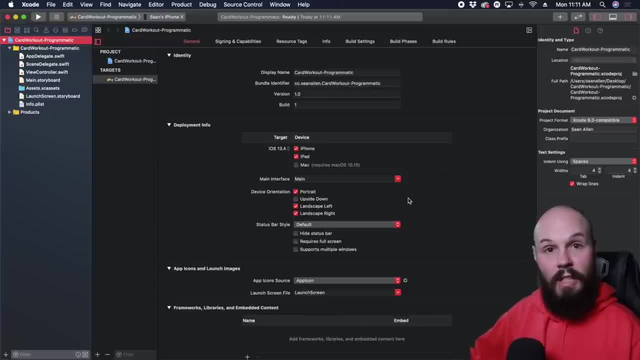 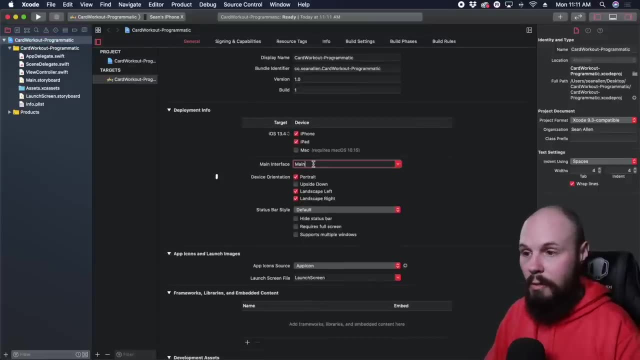 start minimizing this to make some room. so here we are at the general settings, right, and this is where we're going to start removing the storyboard. so here you see, main interface, main. this is main storyboard. so delete that and then hit return. make sure you hit return. 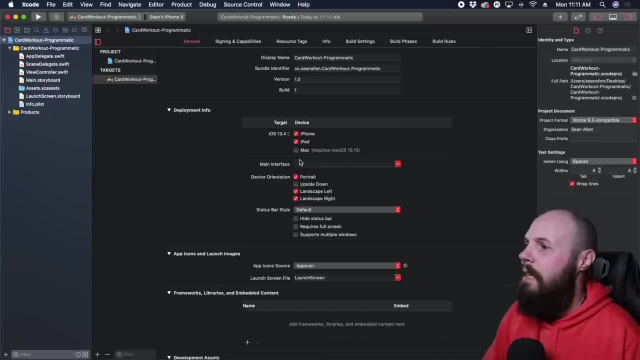 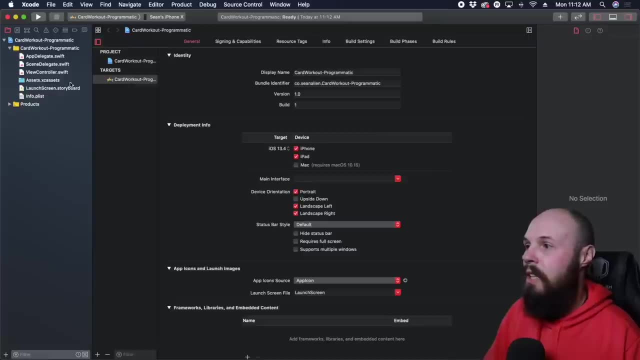 again. that's what actually enters it. hit it twice for good measure. and then now let's click on mainstoryboard and right click it. hit delete. we're getting rid of that thing. move the trash. same thing with view controller. remember that default view controller we get delete. move the trash. 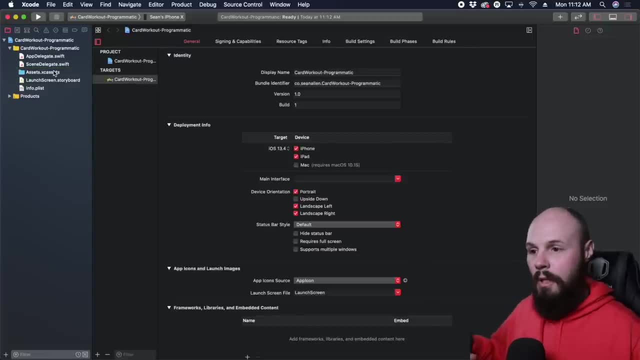 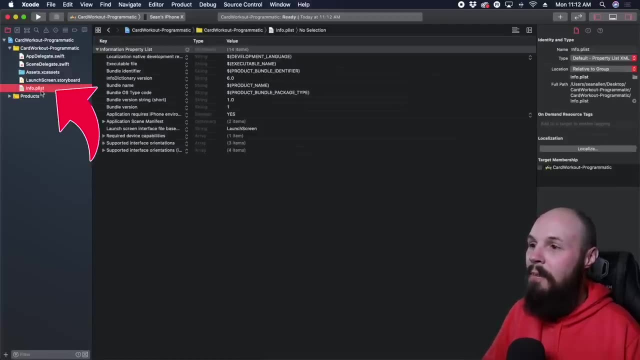 we'll be creating our own, and then the last thing we have to do to like fully rid ourselves of the storyboard on this project is go into your p list right here, and it's best to just search for main. so if you do command f on here, type main. 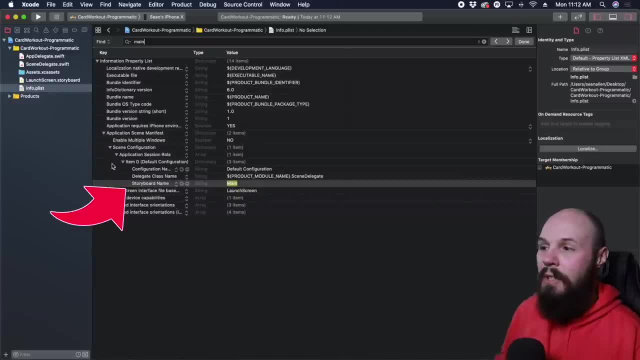 hit return. there you go and you see it. pulled it up storyboard name and you can see i was kind of buried in a bunch of different settings here. that's why it's easiest to search for it. and then next to storyboard name we have this little minus symbol. just click on that minus. 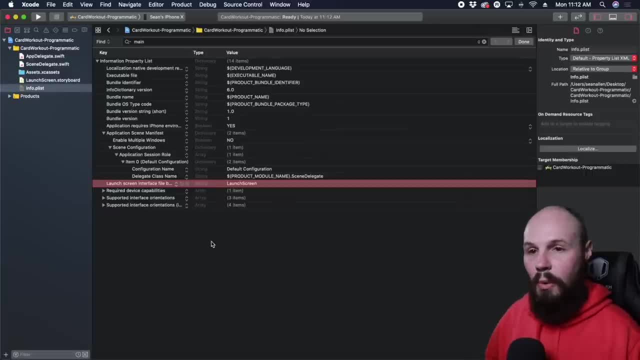 symbol. there you go. we've removed all references to the storyboard because if you didn't delete all those references, xcode would still be trying to look for mainstoryboard and your app would crash because we've deleted it. so now that we're set up to start our project in 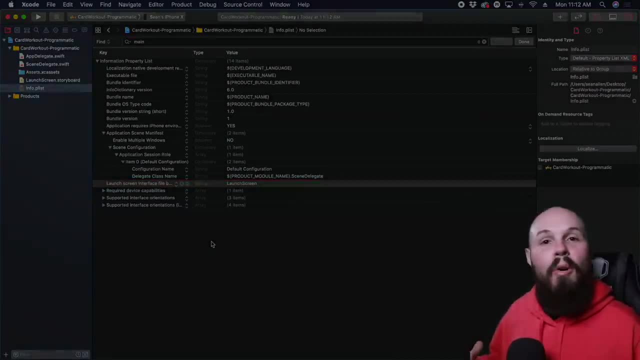 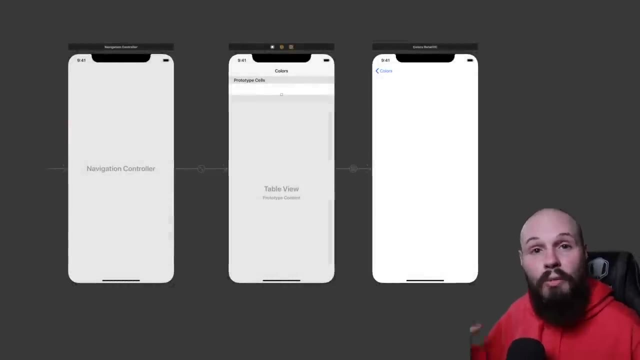 code, because essentially what we're doing. do you remember on a previous project where we had that arrow that pointed to our navigation controller and this was us saying like, hey, this is our initial view controller. we're basically replicating that, but in code, and that's actually a theme throughout. 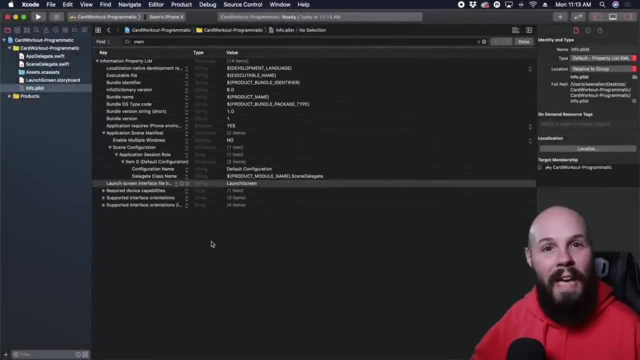 this whole next series of videos. everything we're doing, we're replicating everything we've already done on storyboard, except you just do it via code. so you'll start to see how those things pair. anyway, let's get back to actually uh- creating our initial uh view. 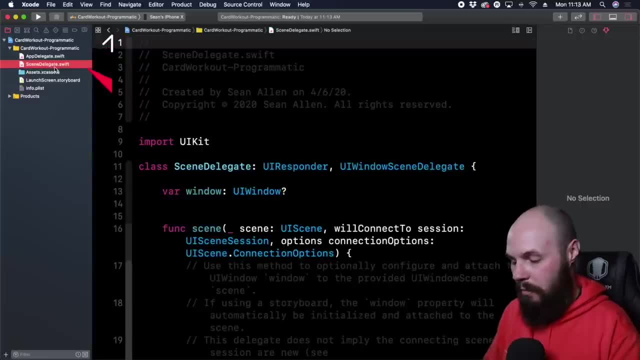 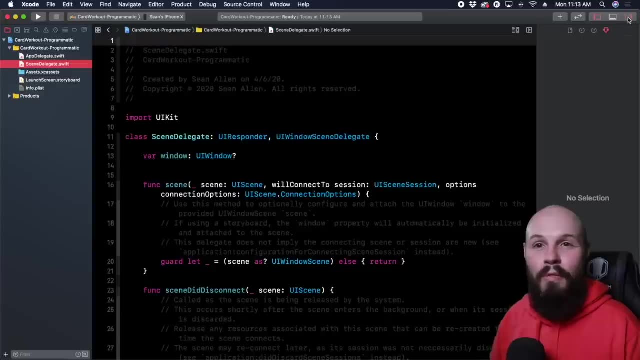 controller. so to do that we go to scene delegate. now let me make my font reasonable here. and the good thing about writing programmatically: get a little extra space. we can pretty much remove this right pane like we pretty much never use it when using code. so the 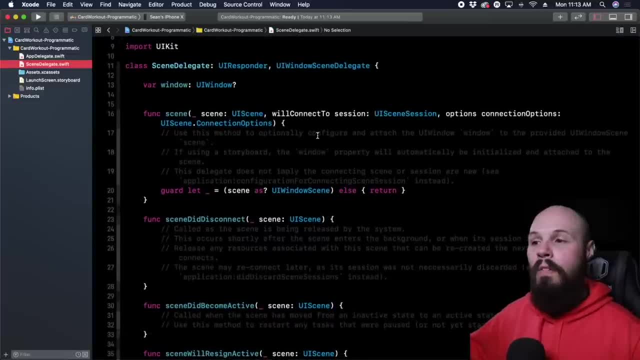 scene delegate. um, i'm going to give you a high level overview of what this is. don't worry if you don't fully understand it. this is way past. you know absolutely the best way to understand beginner knowledge level. um, but essentially what the scene delegate does. uh, and this is new in ios 13, prior to ios: 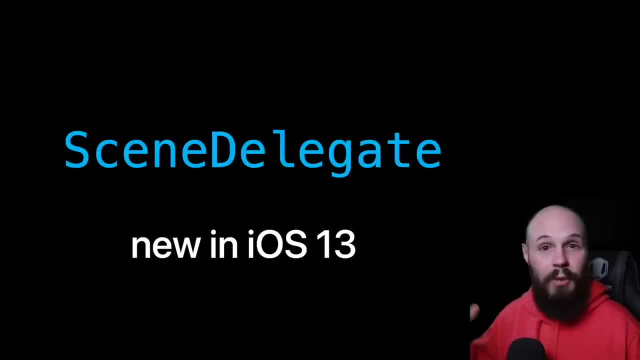 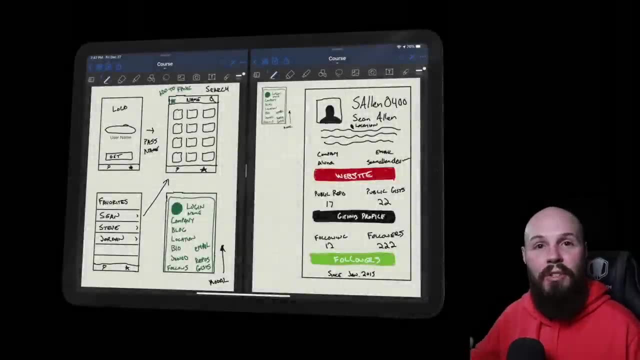 13. this didn't exist. so if you're doing this course and you're still on, like xcode 10 and you know ios 12, you're not even going to see this. but ios 13 introduced having two instances of your app side by side, like windowed mode, and 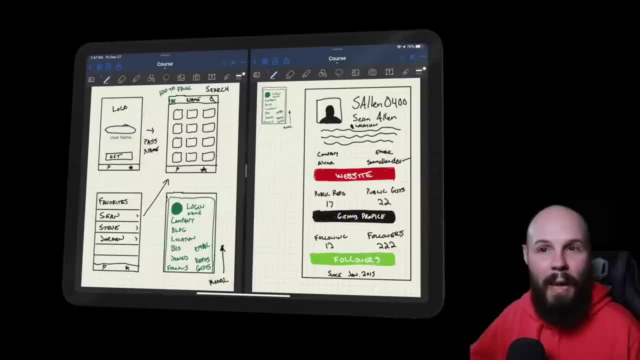 this is relevant on ipads and potentially down the future. you know catalyst apps, where you can have apps on the mac as well. so on the screen you see an ipad with two versions of the app- good- and on the screen you see an ipad with good notes. it's what i use to kind. 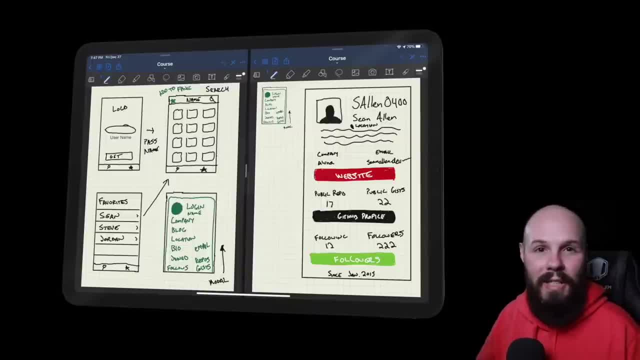 of sketch out some of my apps and you can see it's two instances of the same app side by side. you can test this yourself. open up your ipad, maybe, open up the notes app and pull two versions of the notes app side by side. again, prior to ios 13 you couldn't have two. 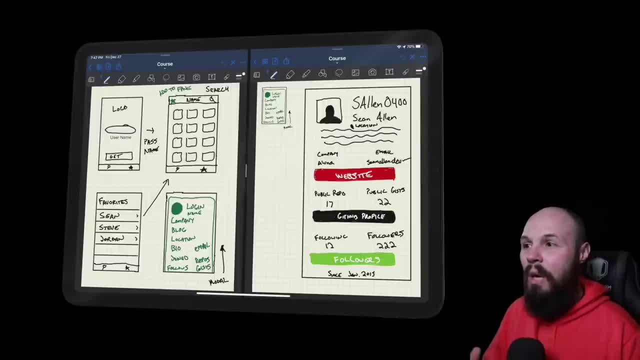 instances of the same app. okay, how does that relate to scene delegate? well, ios 13 introduced what's called scenes, so each instance of your app- again the two that are side by side- is a new scene of your app, because before all we had was this app delegate. so ios 13 introduced 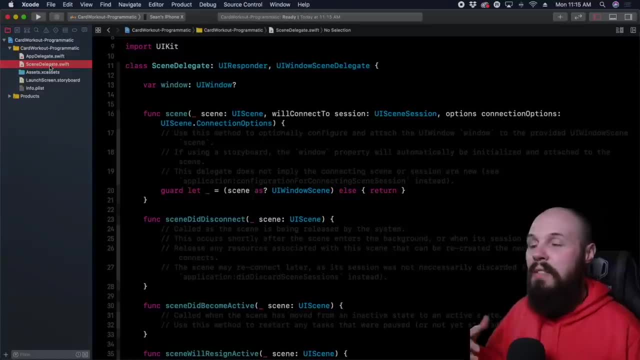 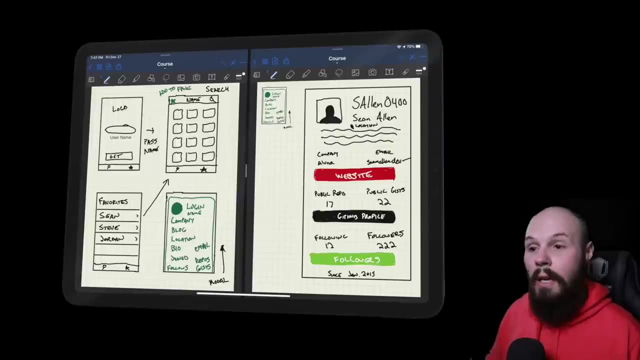 scene delegate right here and you could only have one instance of your app. well, again, scene delegate allows you to have multiple instances of your app again, so you can have it side by side, like you see on the ipad here. that is the high level overview of what the scenes are. 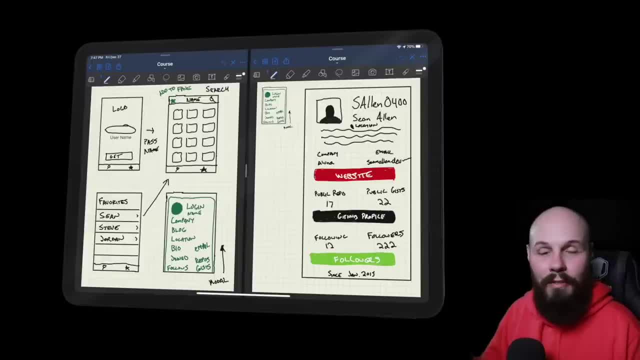 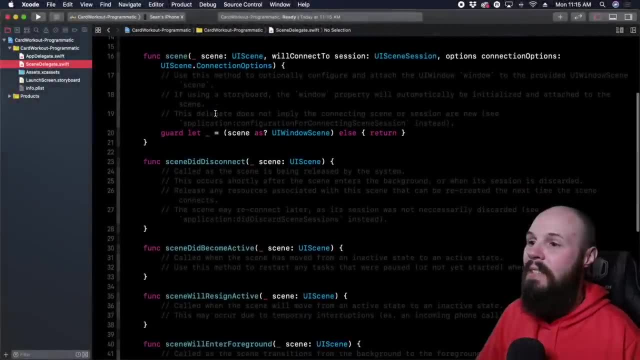 again, no need to go deeper as long as you understand that it just allows your app to have two instances of itself, side by side, like on an ipad or down the line of mac. it's pretty much all you need to know for the beginner, but it is in this. 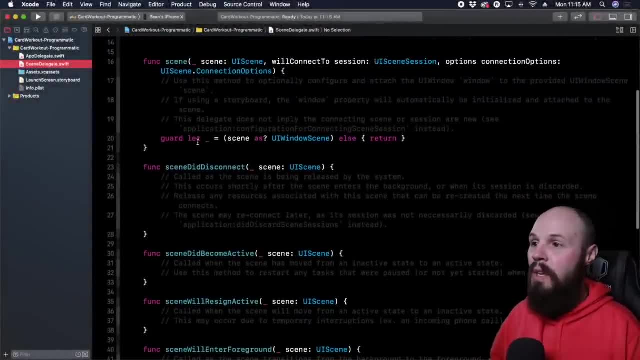 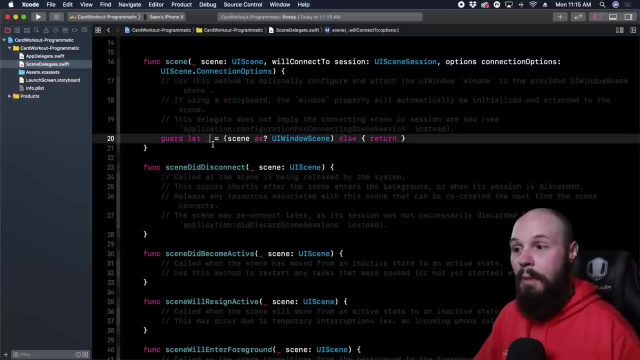 scene delegate, where we're going to write our code in order to show our code. so you see here, guard, let and remember this empty underscore means like there just has no variable name for it. well, we want to give this a name because we're actually going to use uh. 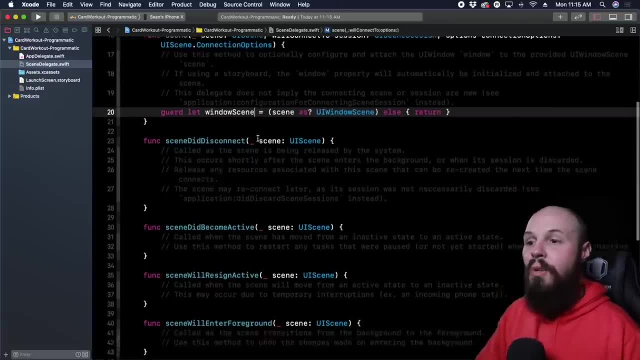 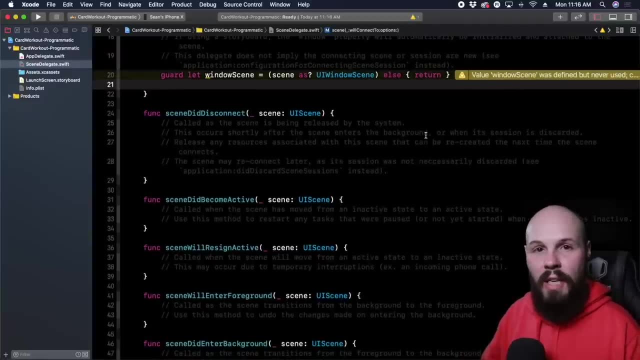 this scene here that we're getting here. so let's create this window scene and i do want to preface: uh, the next bit of code we're about to write here. do not worry if you don't understand this. this is a required step and i'm 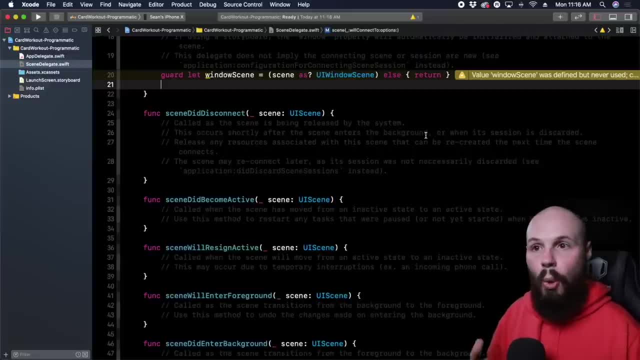 still showing the code so that you have it for reference if you do want to dig deeper or if you want to create your own project later on and you want to do it for reference to come back and look at. but do not worry if you don't understand. 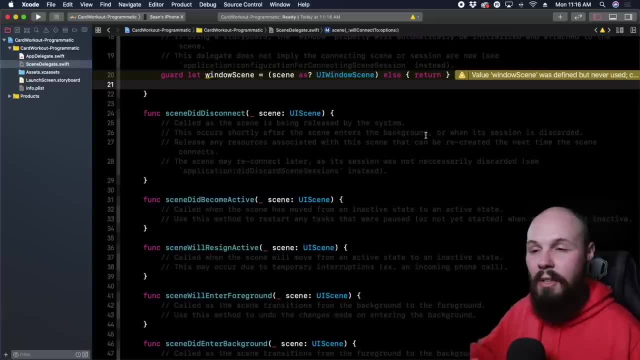 how the ios windows system works and how all these scenes come together. that is way above the scope of these entry level beginner course, but again, it is a required step to get to the stuff that you should know and learn. so we're doing it real quick and 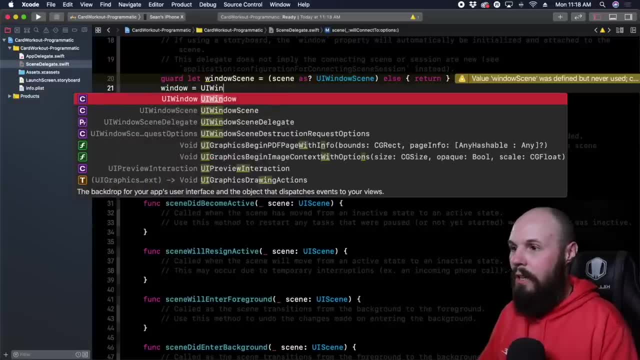 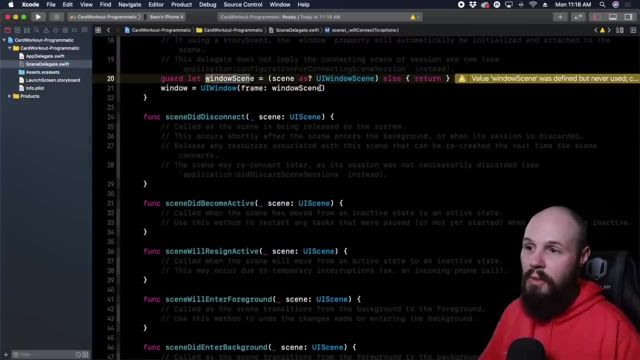 first, we need to initialize our window. so window equals ui window, and we're going to initialize that with a frame of the window scene which we have up here on line 20. that's what we just created, right: dot coordinate, space, dot bounce, and you know what i actually. 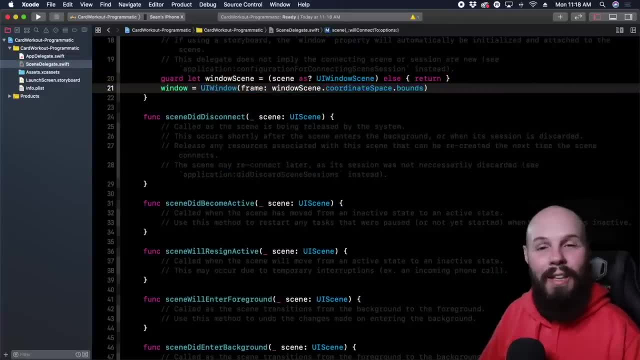 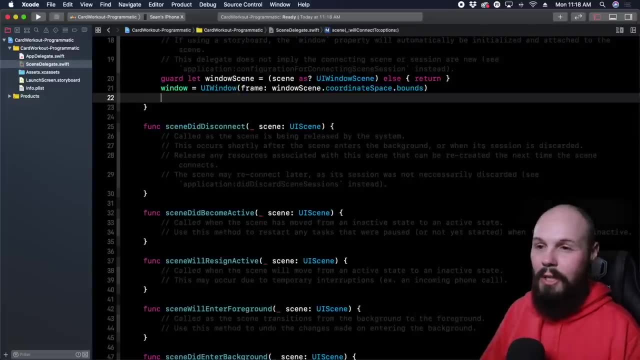 considered just copying and pasting this telling you the high level, and not even like typing it out to avoid confusion, because again i do think this is unnecessary confusion. so again i want to stress: do not worry if you don't get what's going on here. by the way, this window is: 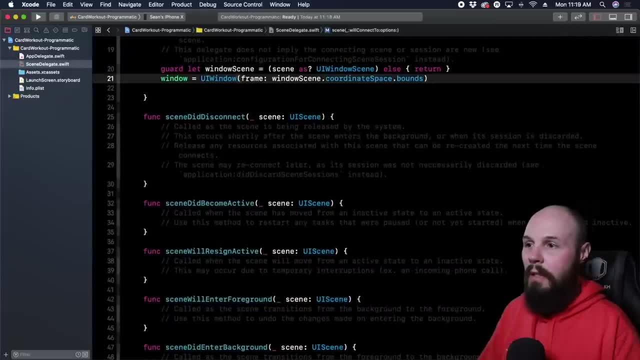 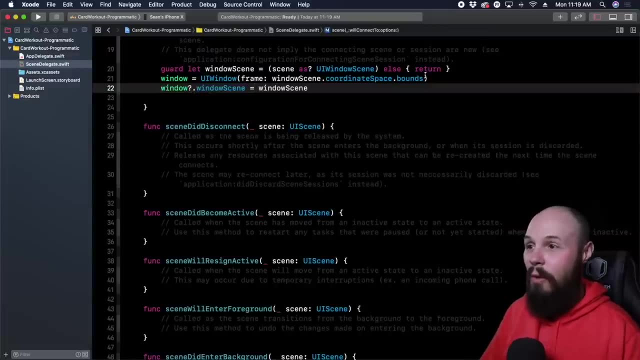 this window variable we get by default from the scene delegate and then now we start configuring our window so window dot. window scene equals window scene. again we're setting the window scene equal to this window scene that we got up here, and then now this is what matters, right. 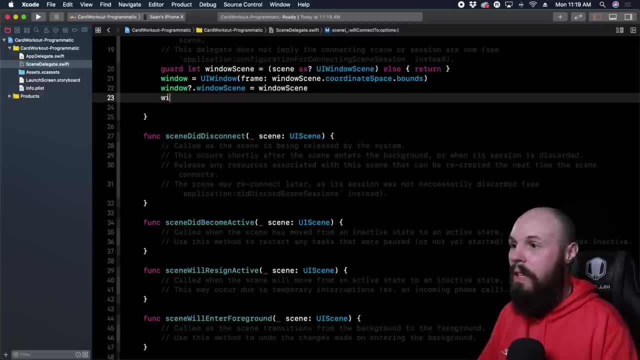 here. this is what you know, you, you should kind of pay attention to. so window, not window, scene window dot. root view controller. so again, this is us saying like here, this is the initial view controller. now, um, we don't have a view controller in our project, right, we deleted that. 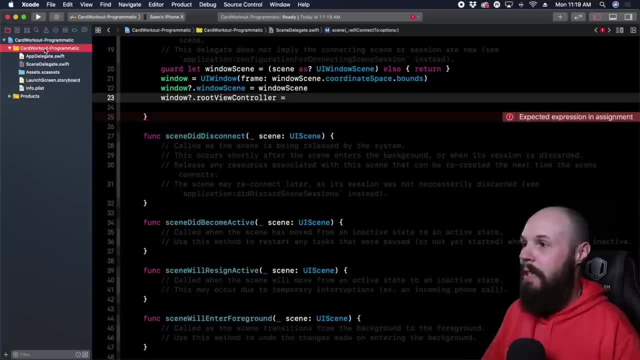 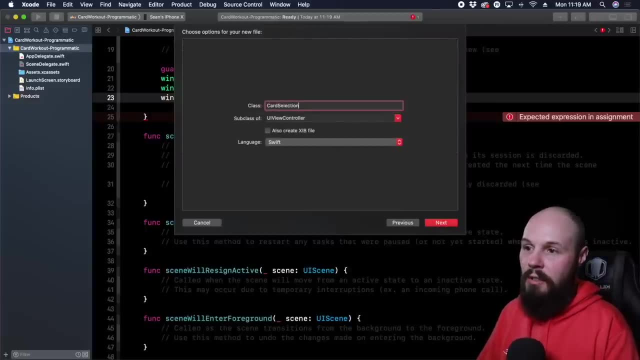 so let's create one real quick. so in our folder do command n- uh- coco touch class. then we're going to create a view controller. hit next- remember, this is the card selection- vc. right, we did that before from our previous project. hit next uh. create it now in our card. 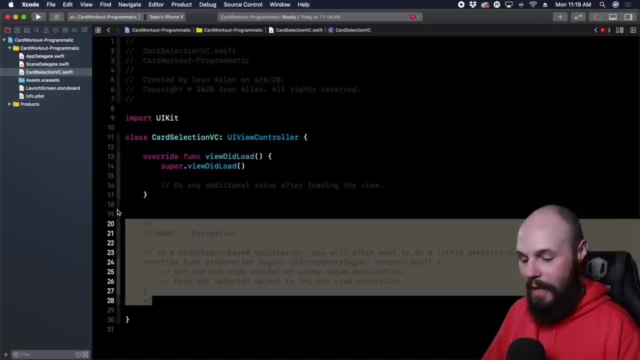 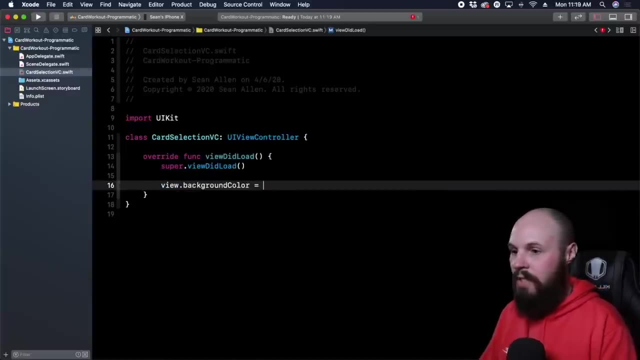 selection: vc again. i always move it up here um just to know that we have this. uh, let's actually set a background color to prove that we're showing this one. so view dot. background color equals dot. um, i've never done dot brown. it's probably look ugly whatever, so dot. 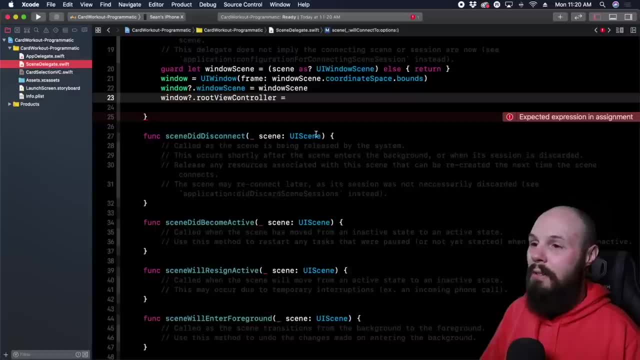 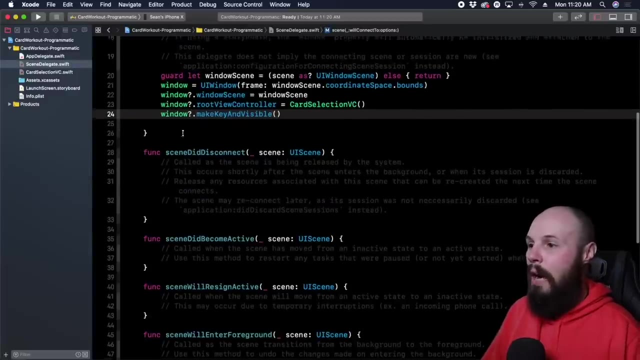 brown and back to the scene: delegate. now that we have that uh card selection vc, we can uh make that our root view controller. so card selection vc, and we'll initialize an empty one. and now the line that makes it all happen is window dot: make key and visible. so now we're going. 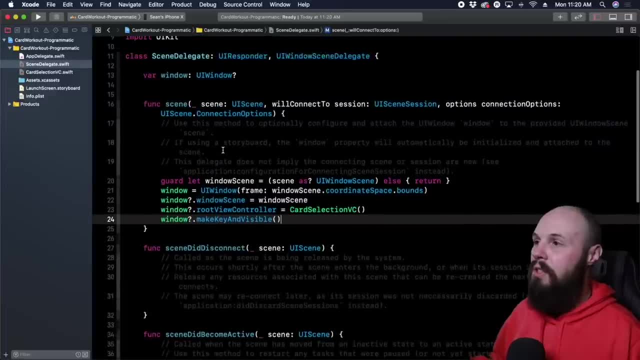 to run this code in our scene. and now, when we run our app, you should see, uh, the brown screen. so let's change this to iphone 11 pro, not my phone. run it, and this should be the setup. we need to show our card selection vc as the initial view controller and here: 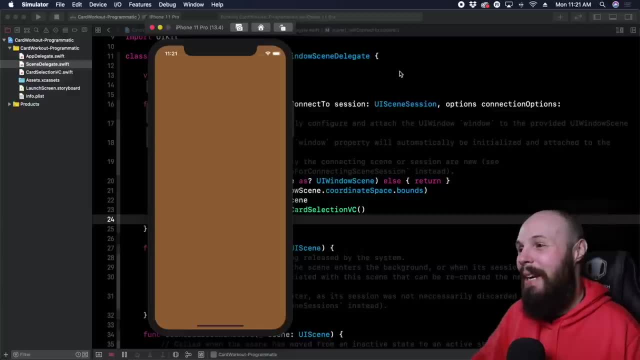 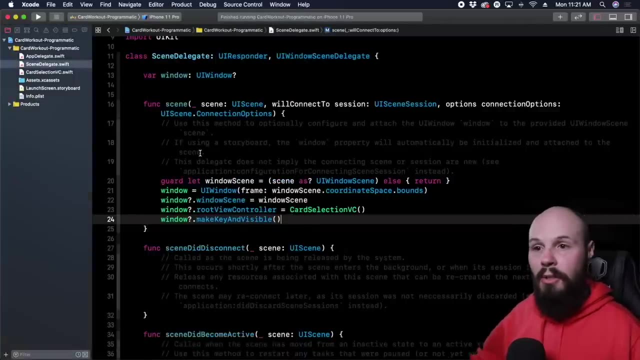 you go, we get this beautiful, beautiful view controller with this nice background. so this proves that we are showing our card selection vc, because our background is brown and this is the initial setup that we need to do to get rid of storyboard and be done with it. now i know what you may be thinking: wow. 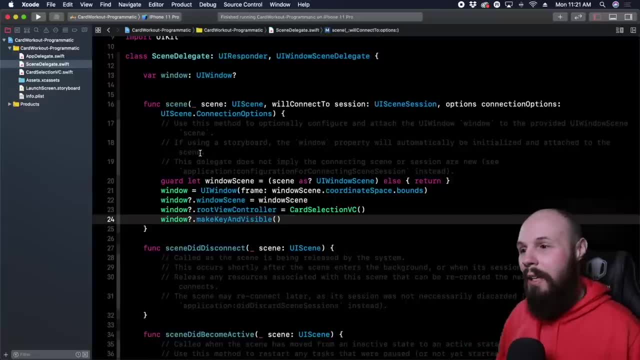 that was a lot just to get our initial view controller showing up. and you're not wrong. right, when you do a storyboard you get all that by default. but again, you only have to do this once when you set up your your project initially, and oftentimes when you're working on a. 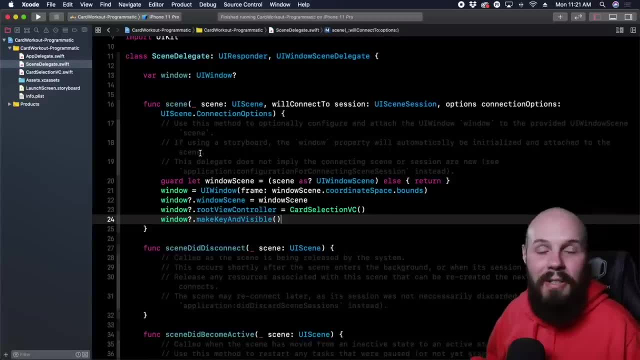 project. you're working on it for months, so you know it took us a few minutes to do this. uh, it is a small price to pay, in my opinion, to get all the benefits of doing everything programmatically throughout your code base and before we go. i do want to point. 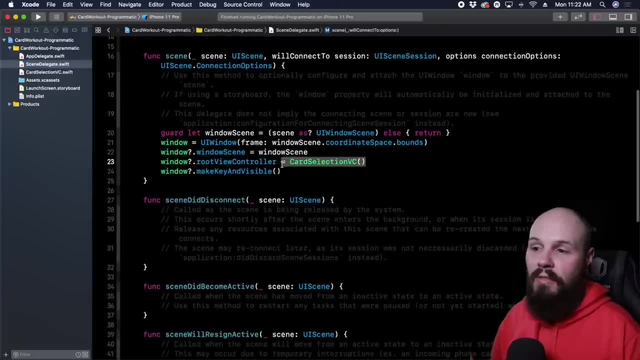 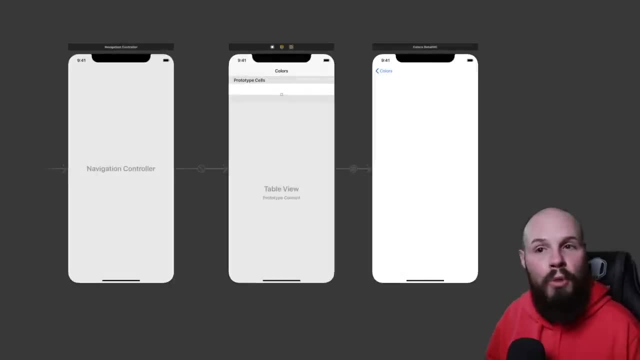 something out about this root view controller. right, we made this the card selection vc. now, remember this is the root view controller. if you go back to our colors table view app, remember our root view controller was actually not a view controller at all. it was the navigation controller. 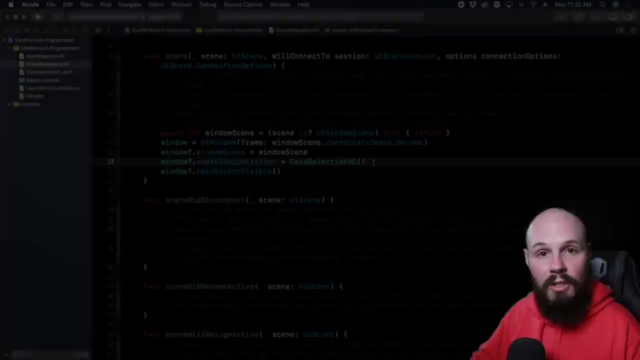 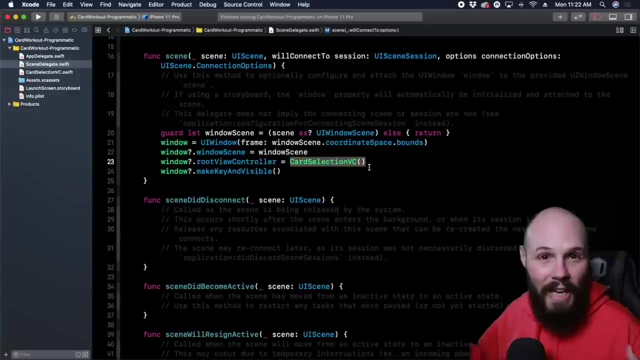 that held our view controllers. so if we were building our colors uh table view app, this wouldn't be a actual view controller. we would be making the root view controller our ui navigation controller. again, that held our view controllers. same thing if you were doing a tab bar at the bottom. 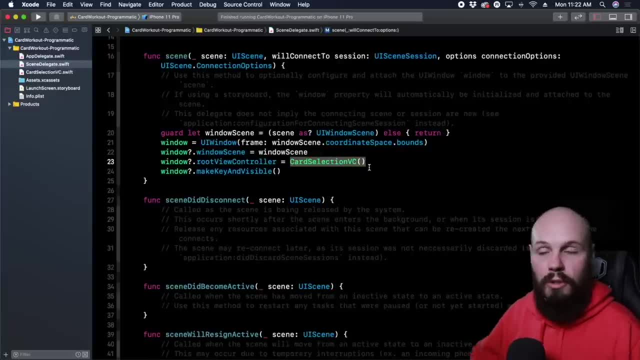 this would be a ui tab bar controller that holds your view controllers. so again, just some clarification. if you are using a ui navigation controller or a ui tab bar controller as your first screen, you want to make those your root view controllers. just quick clarification. and again, one last time. please don't. 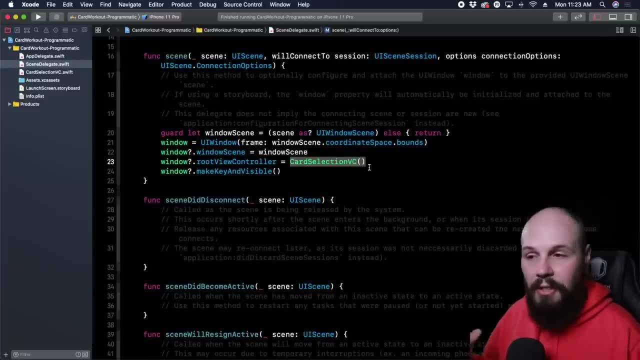 worry if you don't understand this, if all this was gibberish, i don't want you to get discouraged by that. this is above and beyond kind of the absolute beginner, like i've said a couple times before, but i really want to stress it. moving on to the next videos will be a 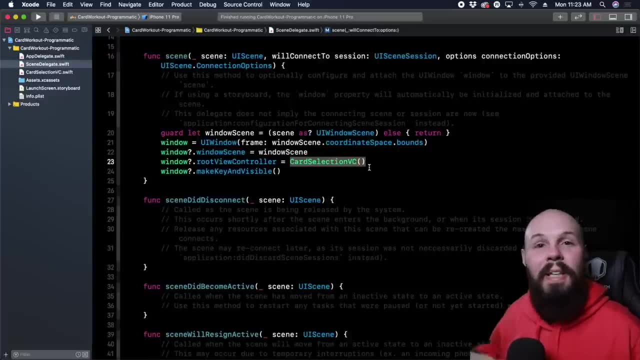 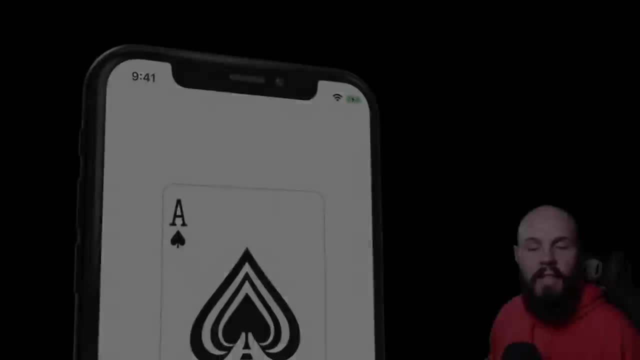 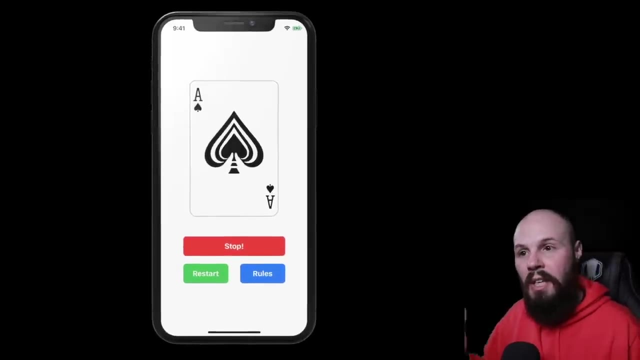 lot less, uh, high level, if you will, and more so beginner content. so again, don't get discouraged, let's move on. in this video, we're going to create a custom subclass of a ui button to handle all the configurations of our buttons right as you see on the screen. 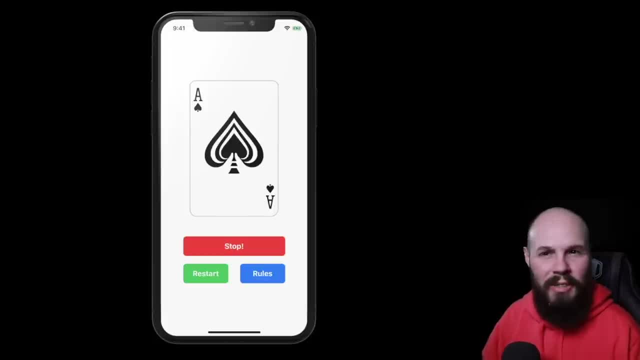 we have the green button. they have rounded corners, the text is white, it's also bold and a certain font size. so we're going to configure all that into a custom button. now, during this video, we're not going to get to see the the fruits of our labor. 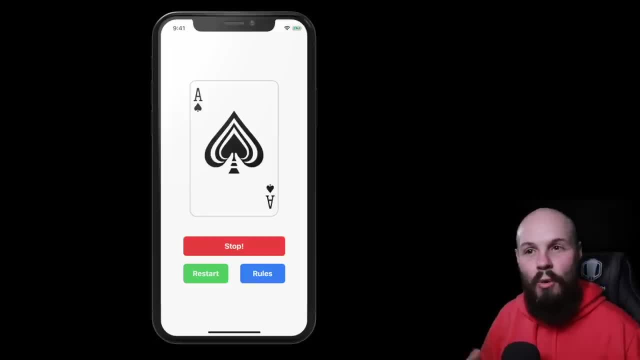 we're not going to get to see our work in action. we'll see that in the next video when we start laying out our ui and you can see how powerful having a, a custom subclass of the ui button is. so where we left off, as you see on. 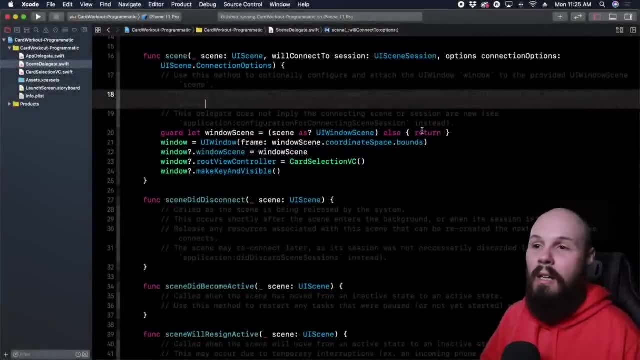 the screen. i haven't changed a thing. this is right where the last video uh, ended. so we need to create a file for our custom subclass of the ui button. so again in the folder for card workout programmatic, do command n for a new file, touch class. 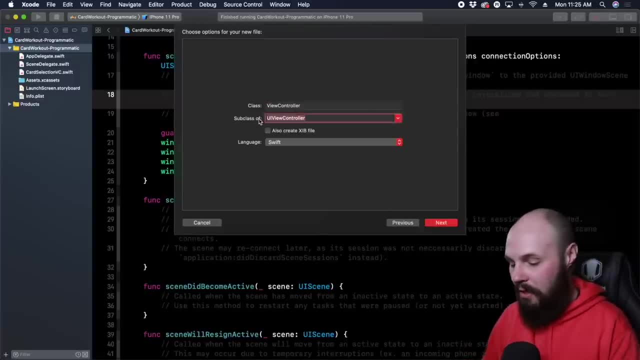 now we've been doing this for our view controllers. now we need to make a subclass of ui button. right, make sure you change that subclass of, so the class we're going to call this cw button. now what does the cw mean? this is a convention that, if you're making custom elements, 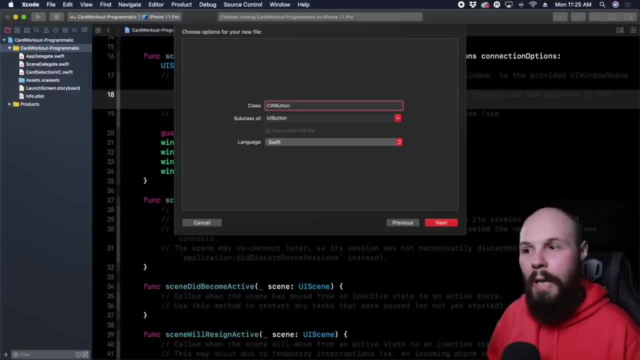 like a custom label, custom view controller. it's convention to add a prefix with your project name. so in this case cw stands for card workout, so this is a card workout button and in a larger project you may have different kind of buttons. so let's say you wanted a certain type. 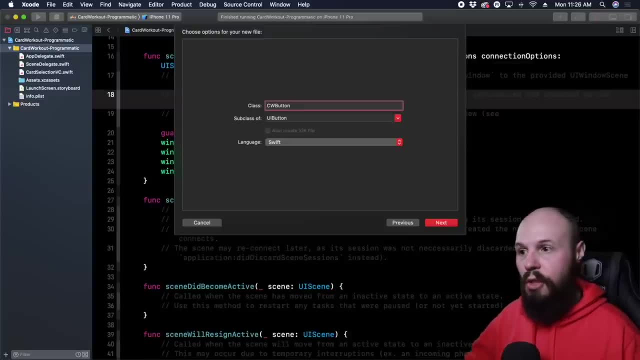 of button that was during your onboarding or your login screen, so you may have like a cw authorization button. maybe you have a cw game button and the reason behind this naming convention is because if you're creating all these custom assets and you just name it button. 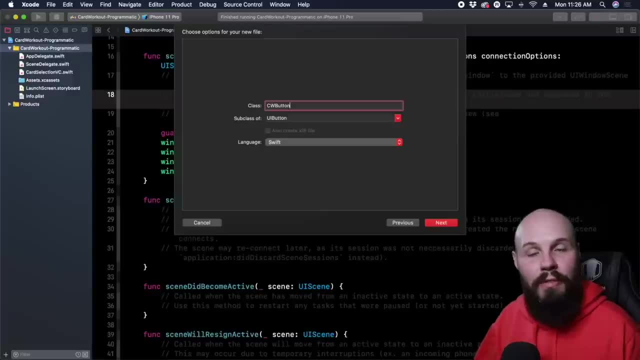 like that's pretty generic. um, however, if you name it with the prefix of your project, in this case cw button, like in the case of facebook, they do fb button or fb, whatever right. so, uh, this will let you know that, hey, this is something we custom created in. 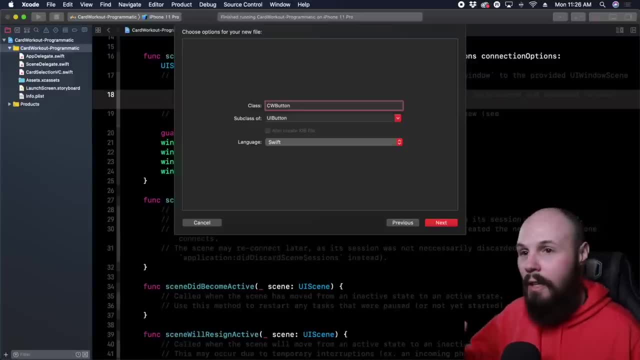 our project. it's not going to be a lot of. it's not part of a library, it's not part of uh, you know, ui kit or something apple developed. this is our custom thing. so, again, adding that prefix lets every user of the code know that. hey. 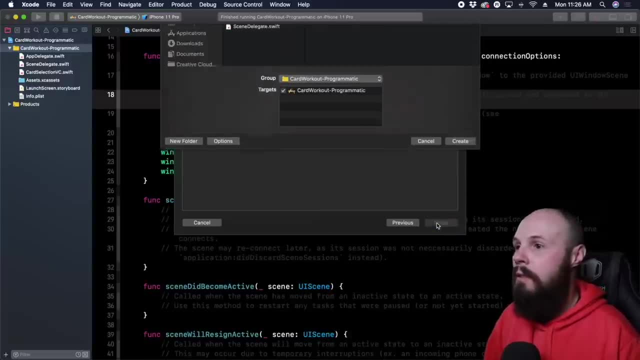 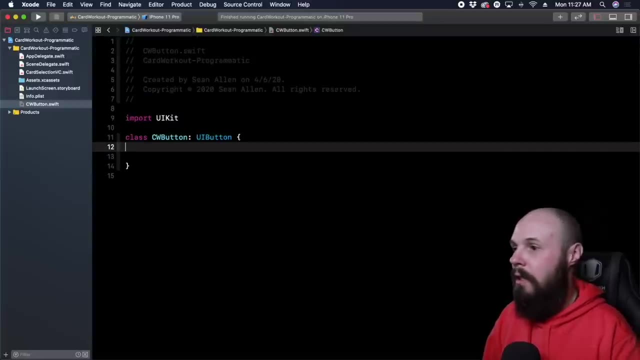 we made this, so name it cw button, hit next uh, create it. now we have our empty button file. go ahead and delete the uh comment here and here we go. we have a fresh start. so let's write our configure function. i'm doing this a little bit out of order. 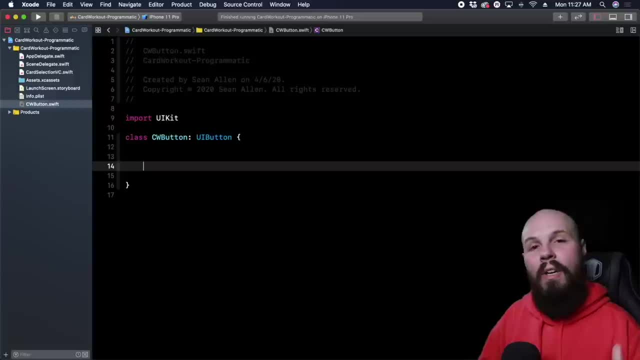 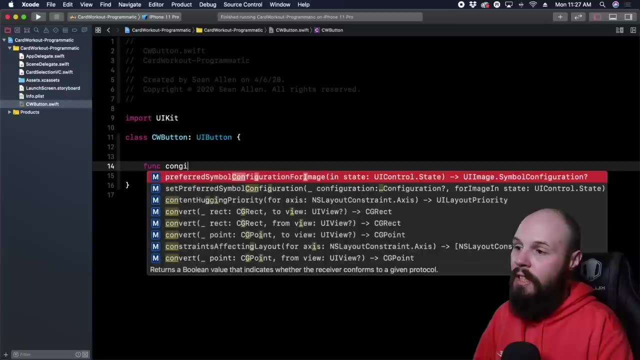 just to let you know, we have to have initializers, but i want to have our configure function done first before we write our initializers um more on the initializers in a second. so let's go func configure. so this is where we're going to um basically. 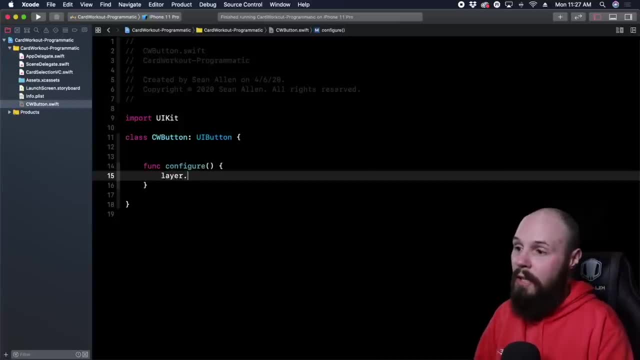 configure the button right. so, for example, we wanted to do layer dot corner radius- remember, equals eight, and it's the same thing we did via storyboard. and then now we want to set the title label: dot font right equals dot system font- remember, that's what we picked. 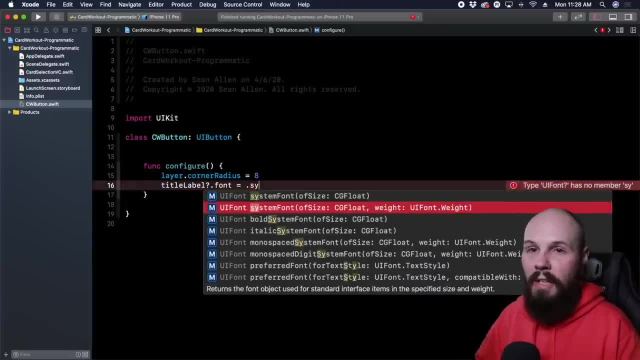 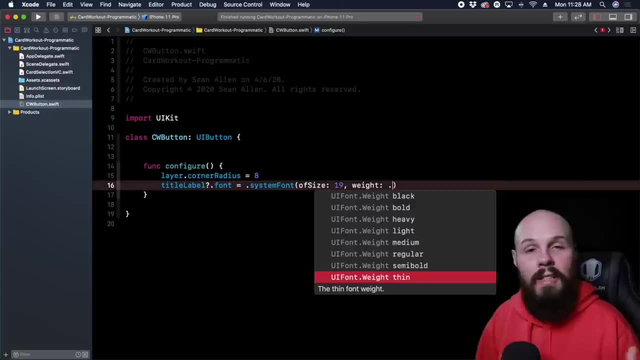 and you can see we can do just of size or we can do of size and weight. so if you're remember, we did a font- i believe it was 19- and then the weight. if you hit dot you can see all the font weights. again, like i said before, we did all this stuff. 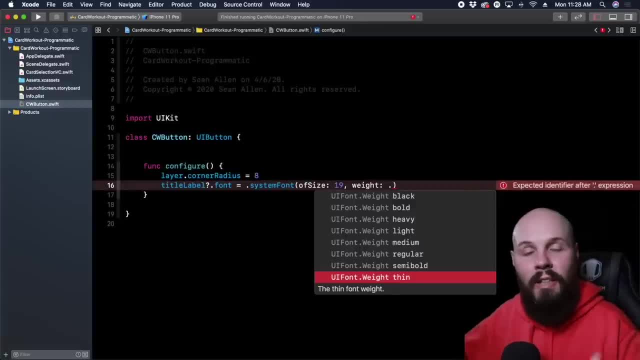 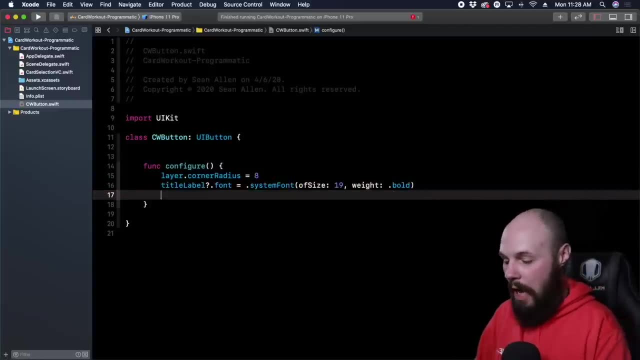 in storyboard. we're doing the same thing. we're just doing it in code and not in storyboard, so hopefully you can see the correlation between the two. so we did bold for the font weight and then now we do set title color down here- the second one. so the color we wanted was white, right? 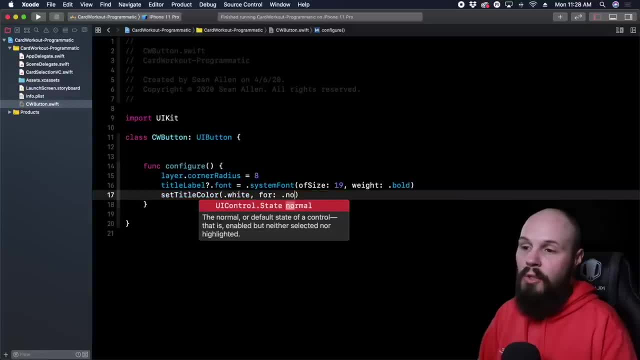 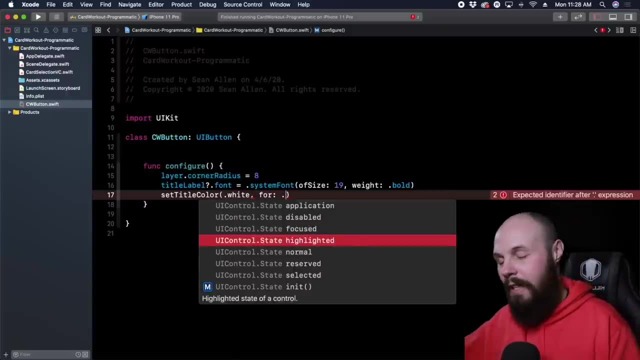 dot white and for control state is dot normal. so you can do and watch. if i do, just do dot normal, you can do. what color do you want if the button is disabled? if the button is highlighted again, that's detailed stuff, 98 of the time you're going to just use. 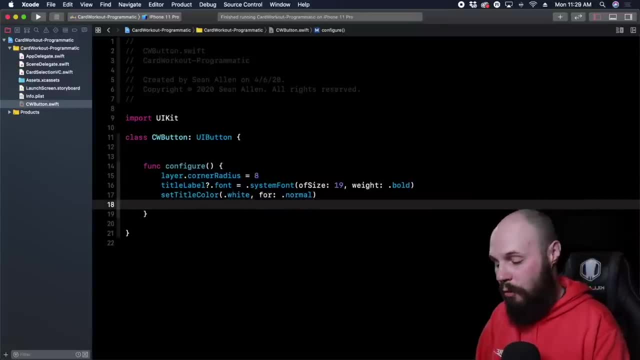 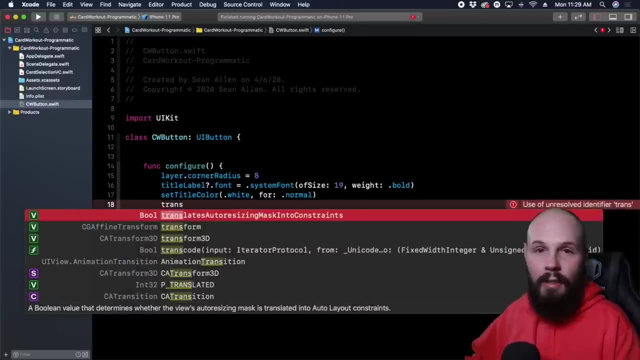 dot normal. now we do something new. this is when you're doing your ui programmatic. so it's translate, it's a mouthful translates: auto resizing mass into constraint. you may hear it called tamic for short. i believe paul hudson started doing that tamic as in like t-a-m-i-c right. 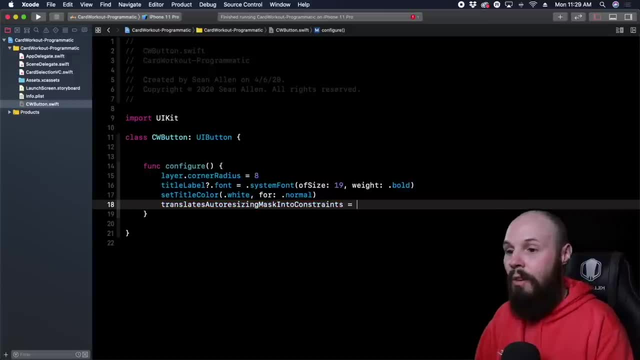 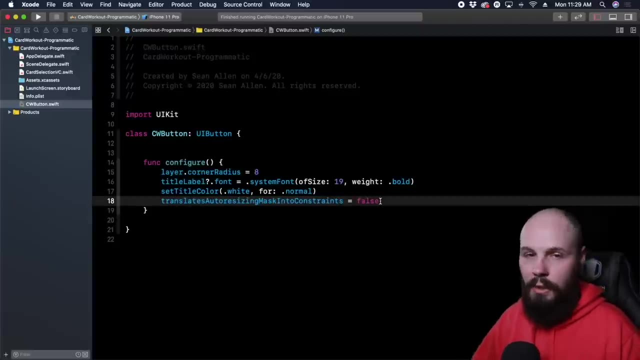 translates auto resizing mask into constraints equals false. essentially, what this line means is is: use auto layout and you'll see we're going to use this line a lot throughout the code base. so you'll you'll get the hang of it. so here's our configure function. so now let's write our 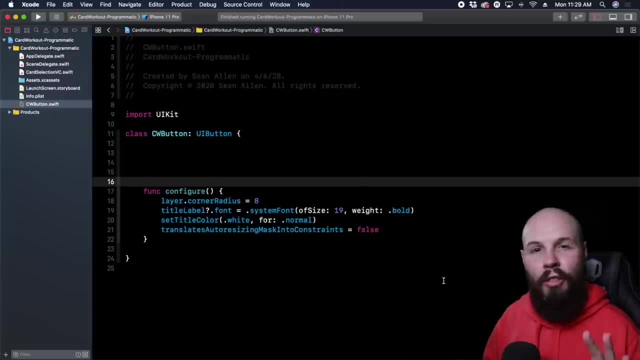 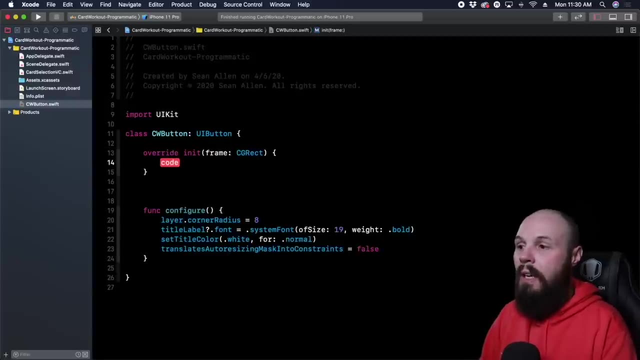 initializers for our custom ui button and we're going to write three of these so i can explain them. so we're going to have the init with frame so this overrides, uh, the ui button init- remember we talked about a subclass- can override its parents class methods. so we definitely want to call. 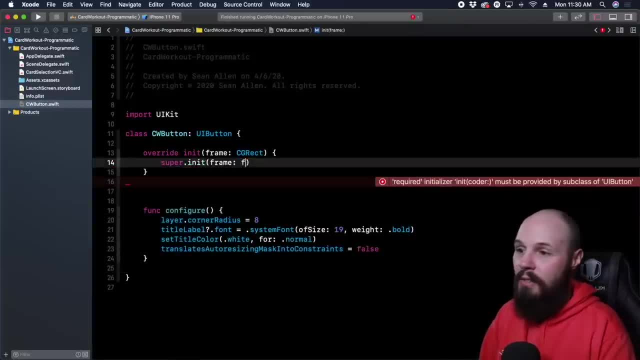 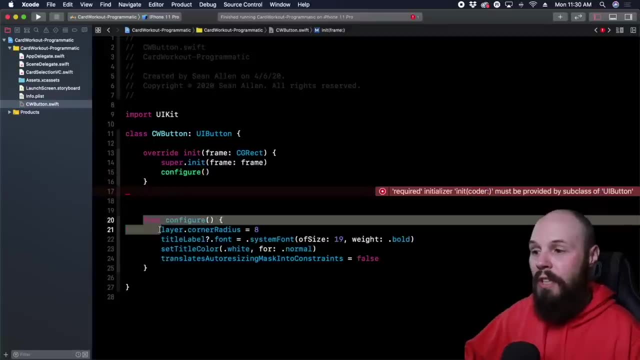 super dot init here with the frame, and then we'll pass in the frame that we we passed in and then here. why we're overriding this init method is because we want to call configure. we want to add our own special configurations right. so whenever we initialize a cw button, we're going to get all the 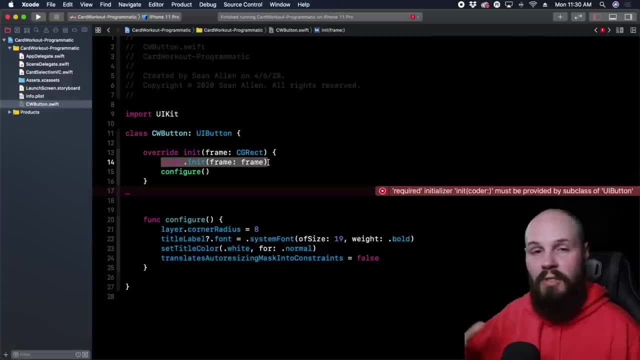 normal ui button initialization. that's why we called super right. that gives us everything apple built within ui button and then by overriding it. you know, in the sub class we add our special little sprinkles on top, if you will, and that's this configure method where we're setting the the corner. 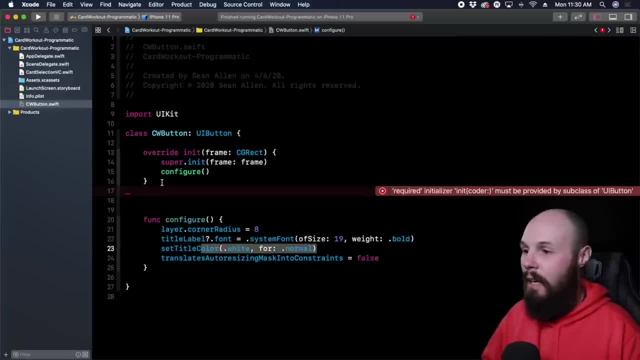 radius. we're setting the font to a certain font. we're setting the font color. uh, it's going to be a little bit more complicated, but that's what we're doing right now. we're going to start to initialize this button and then i'll show you how to do that, but first i'm 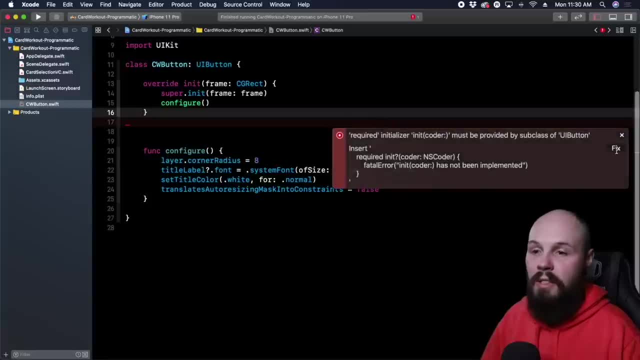 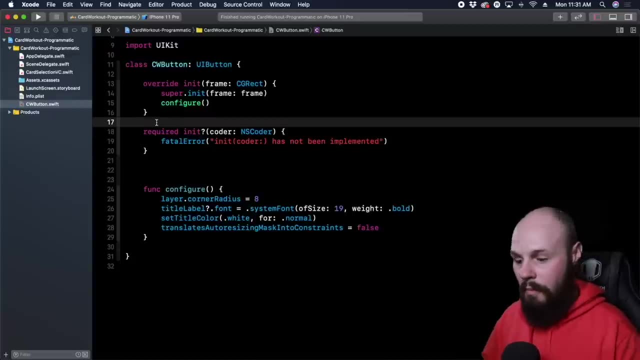 going to show you how to do this. essentially, you're going to want to initialize this button by using your subclass of ui button, so all your sub classes in code are pretty much going to have to have this. and essentially what this coder and it is is, if you initialize this button via. 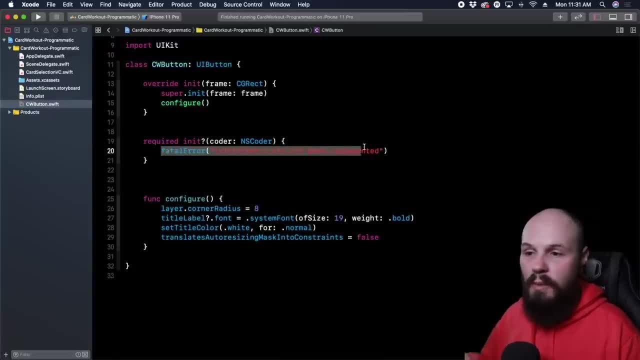 storyboard. now xcode makes us put it in there, but we're just going to keep this fatal error that comes by default because we don't even have a storyboard. so in our project it's impossible to initialize a cw button via storyboard. but that's what this initializer is for now, maybe. 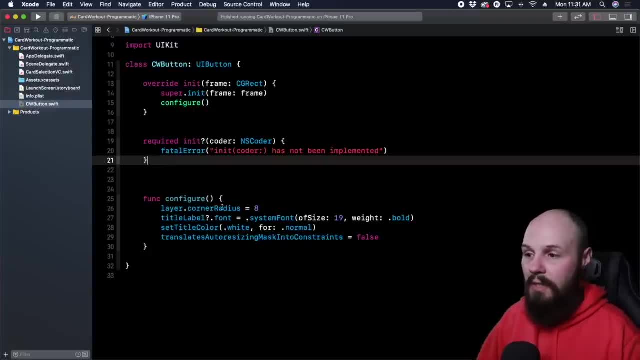 something is missing, right, our cw buttons. yes, we have the corner radius, yeah, we're making our label of a certain font, our label is a certain color, um, but we're missing, like, what is the background color of our button? what is the? what is the title of the button? say, right, stop, reset rules. well, 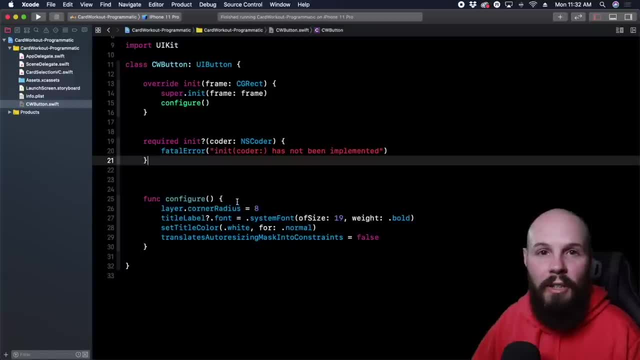 those are different in between buttons, right? so we can't put those in our configure, because that means every button will have the same title or every button will have the same background. so what we can do is create a custom initializer that takes in a background color and a title. 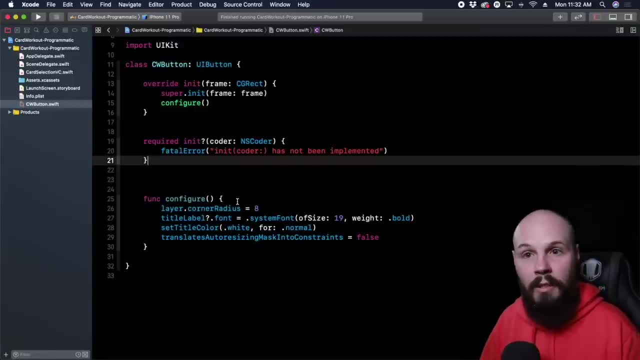 as a parameter when we initialize the cw button, so that anytime we create a cw button we have to give it a color and we have to give it a title. that way we can change the background color and title dynamically. so let's create that again. we're just going to create an init and we're 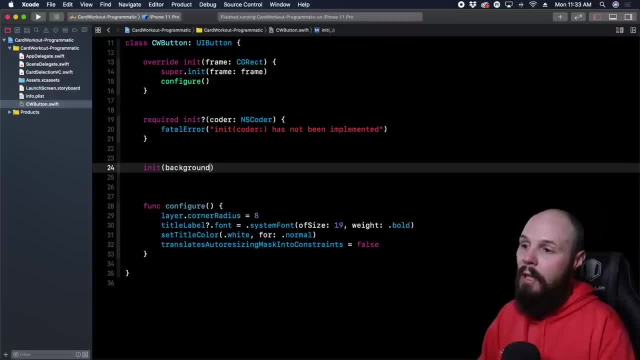 going to pass in some parameters. here we're going to pass in background color and that is going to be of type ui color again. this is just like creating a function where you're passing in parameters and we want to give it a title which is of type string. so now, anytime we do, an initializer. 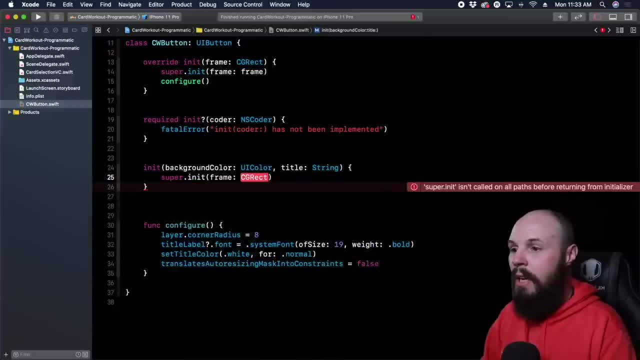 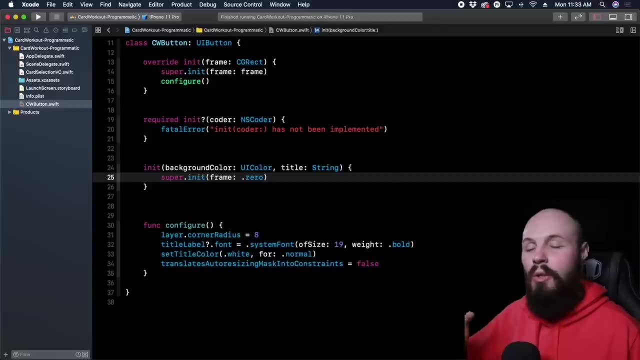 remember we want to call the super, so super dot init with frame, and then the frame we're going to pass in just do dot zero. essentially this means like: so what a frame is is just like you do the constraints right. it needs to know a height, a width and an x and y coordinate. and actually let me initialize a frame so you can. 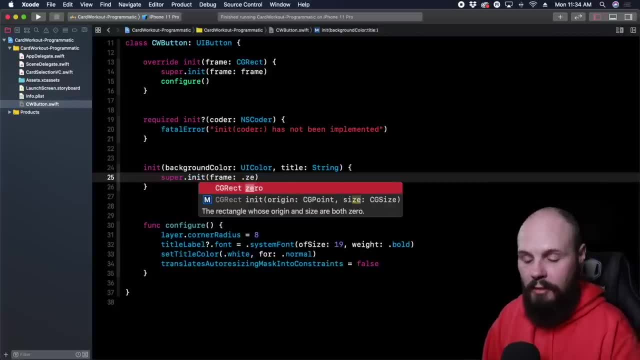 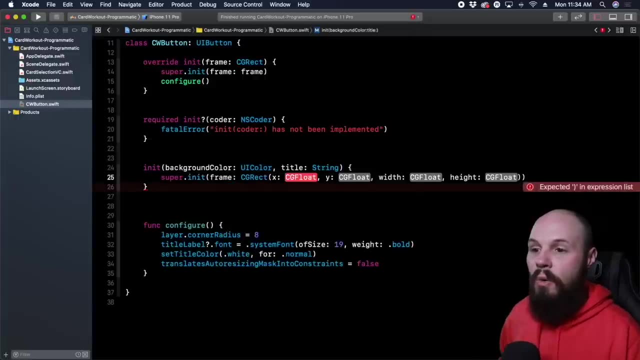 see what i'm talking about. um, you'll see here. uh, it takes in a cg rect, so rect is a frame. so do cg rect and you can see the initializer. uh, like i said here, x coordinate, y coordinate width and height. so by doing cg, uh, i'm sorry doing. 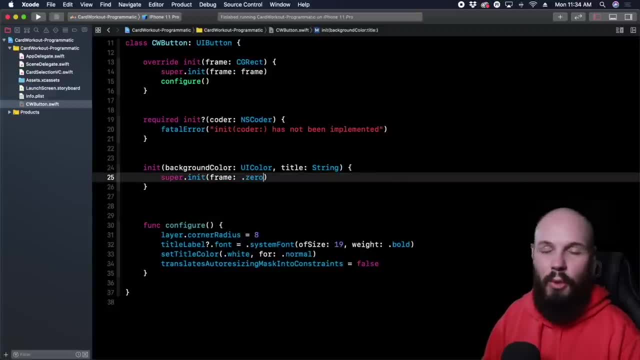 frame dot zero. you're just putting in zeros all of there. this is kind of like a shortcut not to have a boilerplate, and the reason we can have zero height, zero width, zero coordinates is because we're going to lay this button out using constraints, uh, in our view controller, in a later video, uh so 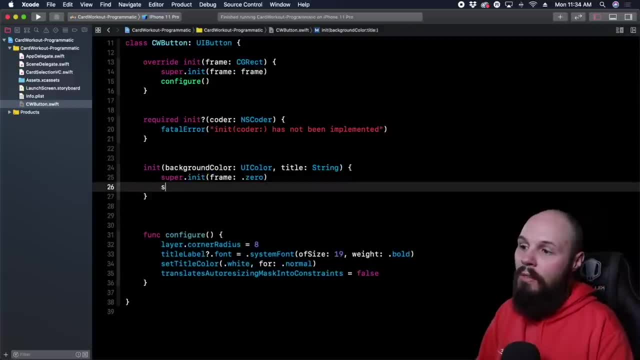 anyway, now let's start configuring this where we can do self dot background color. now again, remember we have to put the self in front of it, because this background color, that's blue, is of the same name. that this is right, like i could have just said color and not named it the same, and then 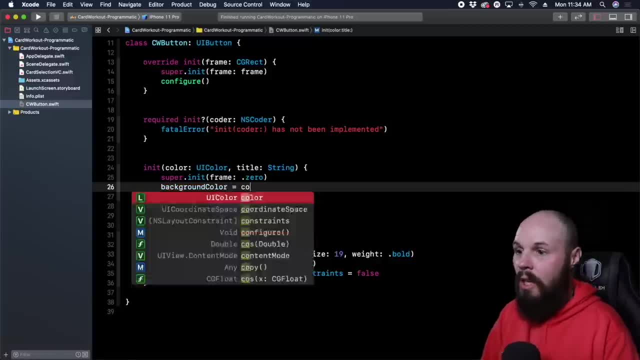 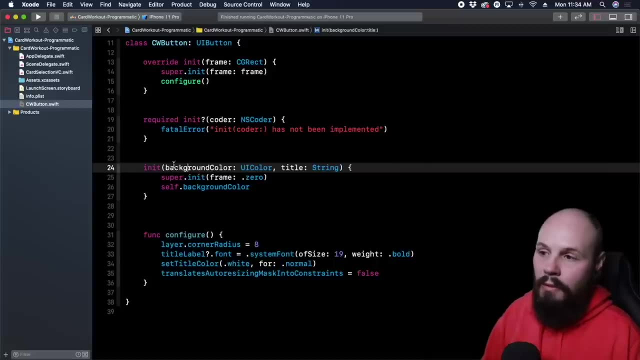 i wouldn't have to do self, you know, so i could just do. background color equals color, right, but background color. i'm just going to command z back to what i had. background color is more informative. just know that if your parameter name is the same name as the actual property on the button you have. 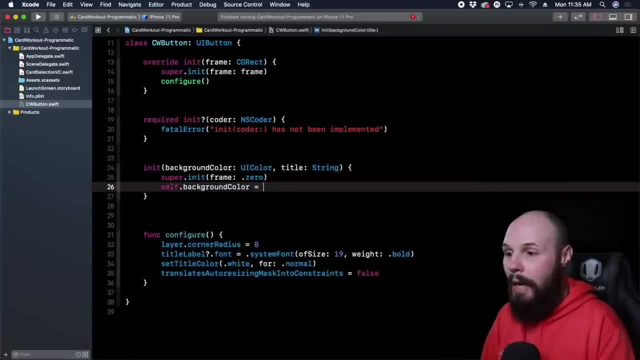 to put self in front of it. so that's why you see that. so now we're going to do equals background color and you'll see this one will be white, which means it's the parameter. the one in blue means it's actually the property on the ui button, or cw button in our case. so now we're setting the. 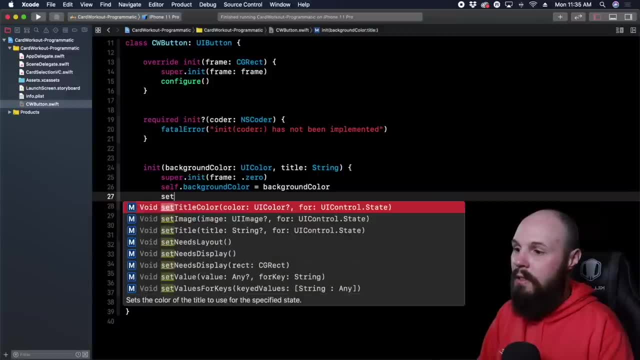 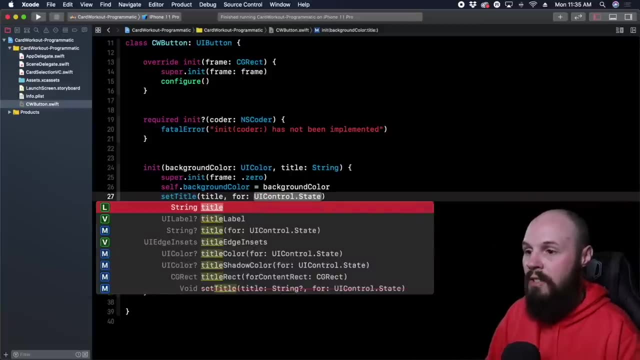 color we're passing through and now we can do set title down here and it takes in a string. well, we have this title here that we're passing in, so title again whatever we pass. and then for control state dot, uh, normal. so this is our custom initializer again when we initialize the cw button. 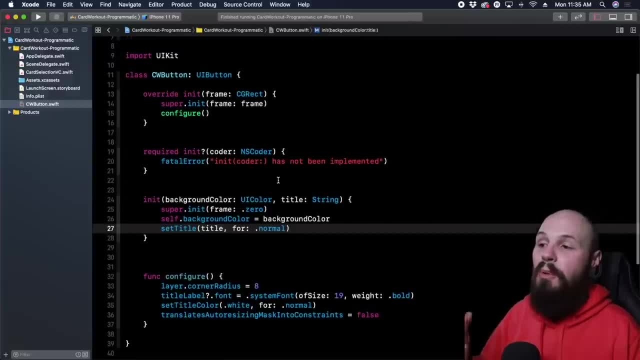 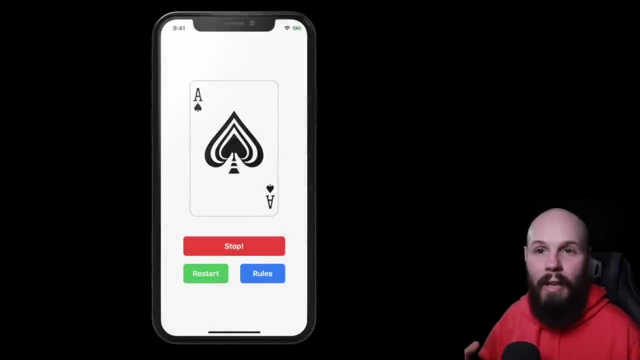 we'll have the choice to initialize just an empty one, or we'll have the option to initialize it with a background color and a title, and you're going to see that in action in our next video when we start laying out the ui for our card selection screen. that you're going to see in our next video. 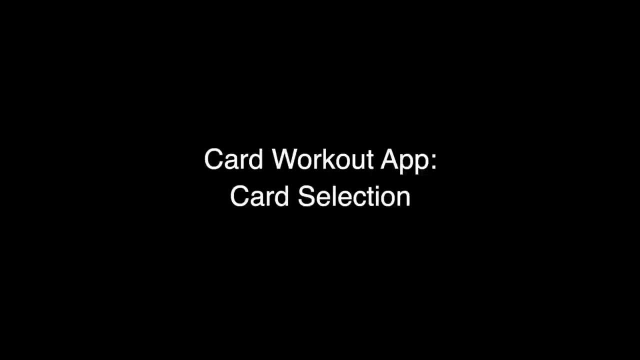 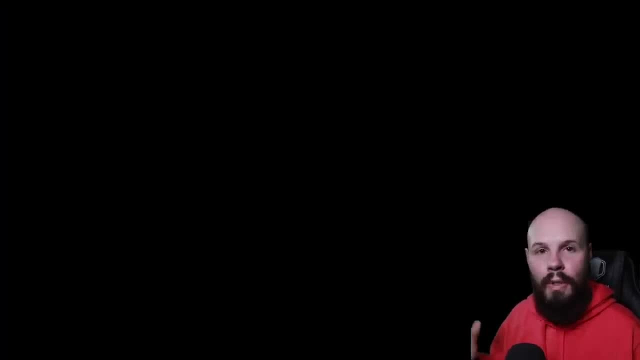 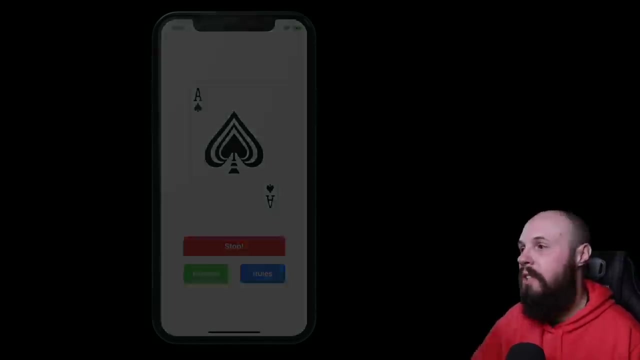 you see here. so let's keep it moving all right as usual, right where we left off from the last video. in this video we're going to lay out the card selection screen that you see here on the screen again, just like we did in storyboard, except we're going to do it via code. so let's actually move this cw button up before i forget. 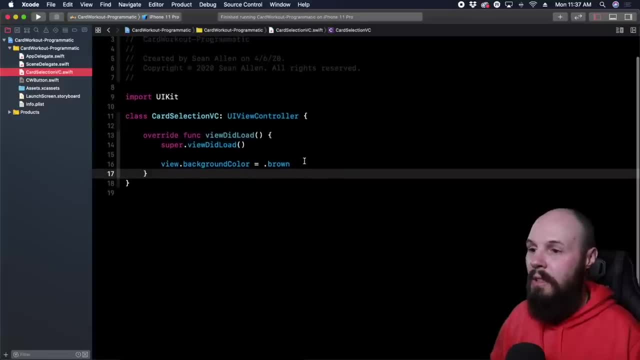 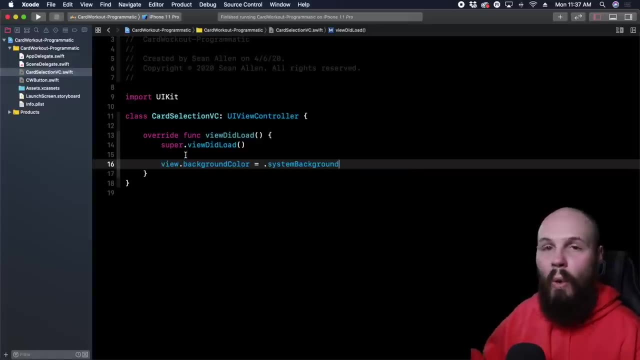 click on your card selection, vc. here we go. we have an empty screen. let us not make this dot brown, let's do dot system. uh, background. and remember, if you want to make this background system, background is what gives you white in light mode and black and dark mode. that's why we do. 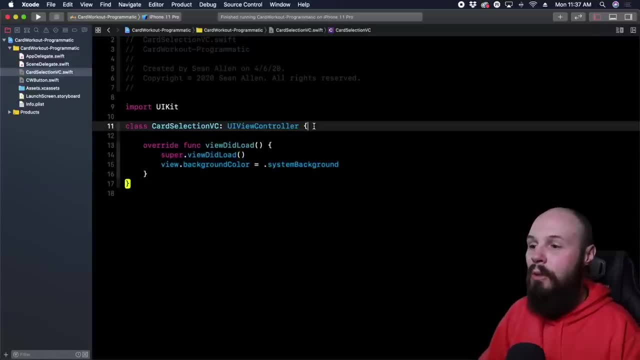 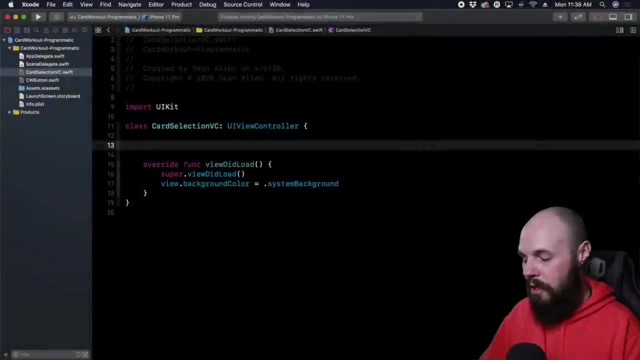 background color equals system background. so the first thing we want to do is start creating our elements. right, we have the ui image view and the three buttons again, like you see here on the screen. so let's create those in code we can do. let card image view, again kind of similar to outlets. 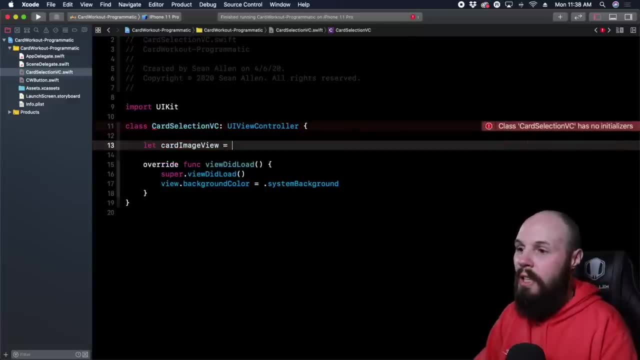 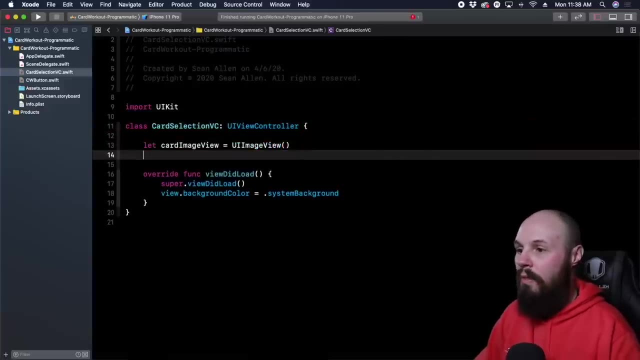 not quite, but you'll see the similarities card. image view equals and this is just an empty uh ui image view here, remember, we drag the image view onto the screen. uh, now we want to make this a button. right, we have our image view. now we need the three buttons, so let stop. button equal: uh seat. 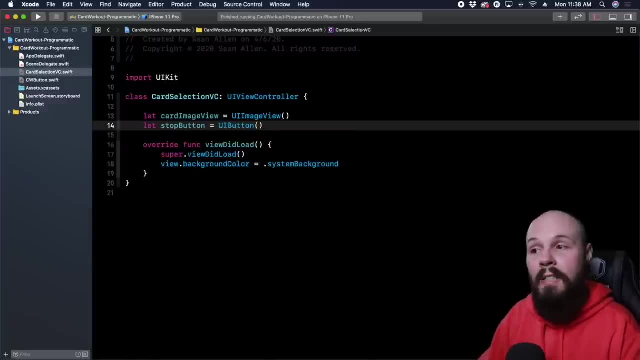 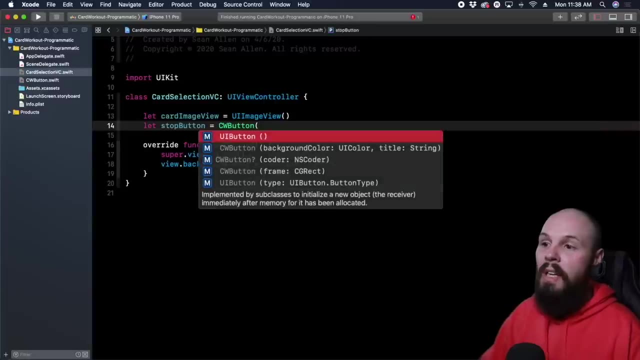 not ui button. right, that's what you may be thinking. no, we created a custom button, remember so cw button that we just created. now watch when i get the initializer here. i do open parentheses. now you can see i can just uh, initialize just an empty cw button. this will call our configure. 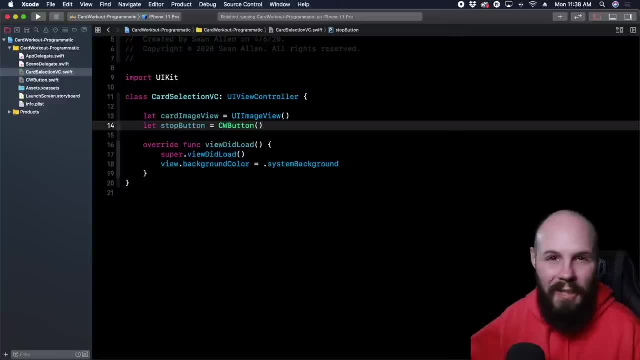 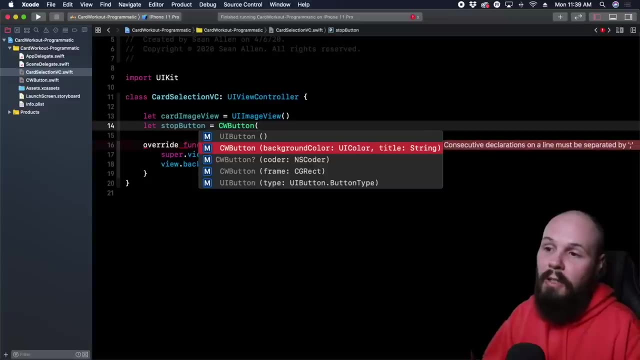 method, but it won't have a background color set and it won't have a title. so we don't really want to do that, but we have the option to. if we want to create a background color set, we can do that. we need to. so now, if i do the open parens and you can see i have our custom initializer right here. 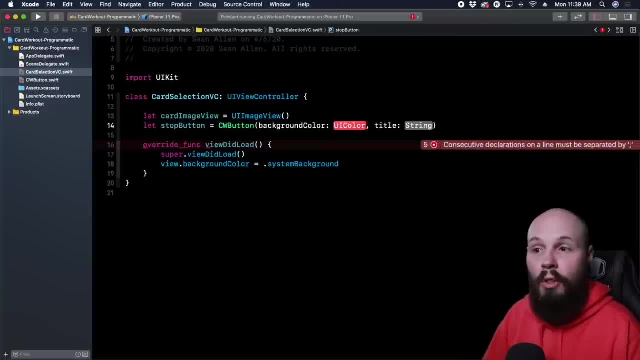 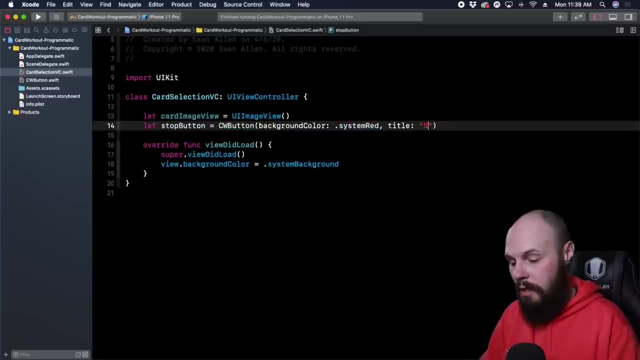 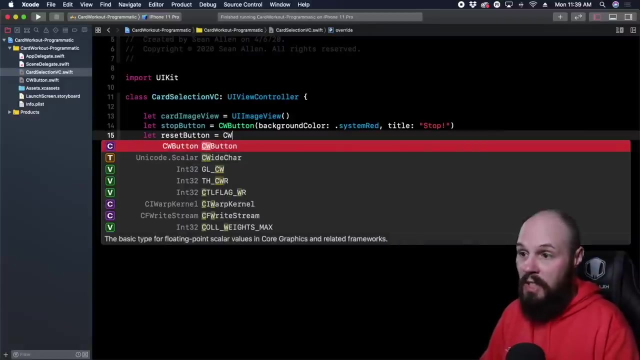 that takes in a ui color and a title. so now we're going to initialize our three buttons like this. so the stop button was dot system red, as you see here, and the title passing a string was stop- exclamation point. and again same thing for the rest of our buttons. so let's reset button equal cw. 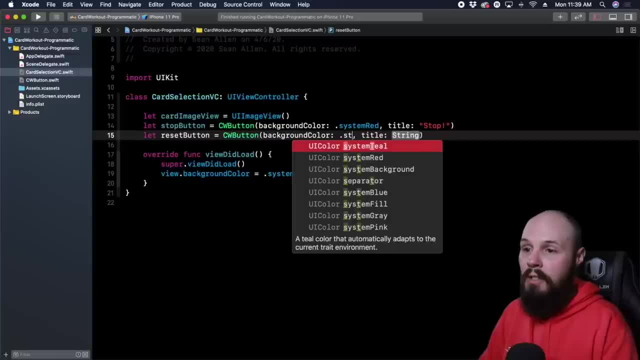 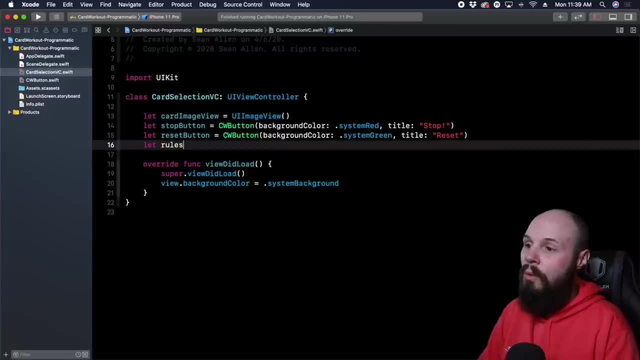 button again with our custom initializer of a background color: dot system green. the title here reset. there we go, there's that button, and let rules button equal cw button with our background color. this one was dot system blue. we have the auto complete there and again the string title: uh, rules. so there are. 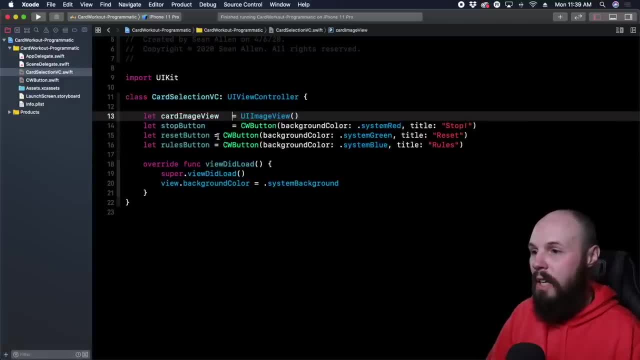 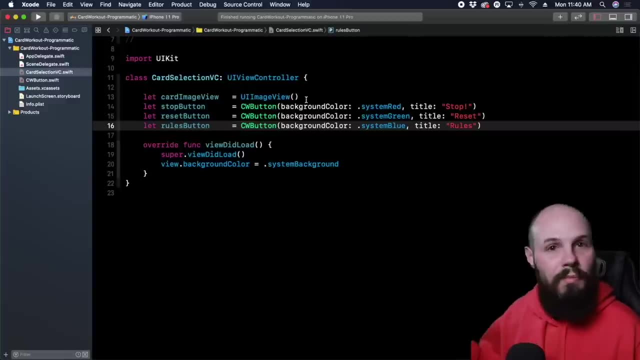 three buttons. now, like i said before, i like to line up my equal signs. uh, this is a style. some people don't like this style. i think it makes things look nice and neat. there are pros and cons. do it, do it if you like, don't do it, it's fine by me. so now we have our objects created. 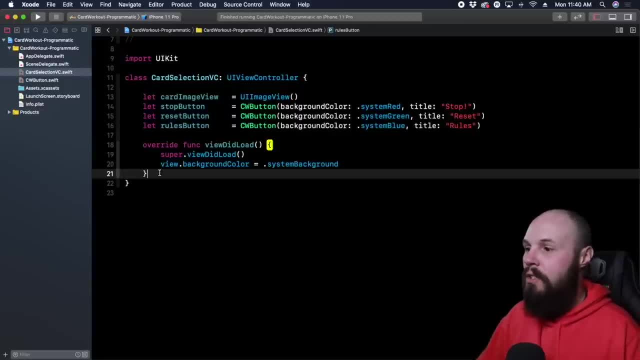 the next step is to configure and layout each object, so i'm going to break this out into separate functions. how you organize this code is very subjective. some people like it a certain way, some people like it another way. i'm going to break it out into extra steps, just so it's easier to. 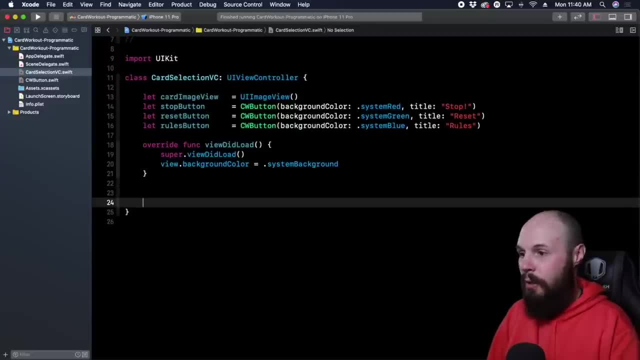 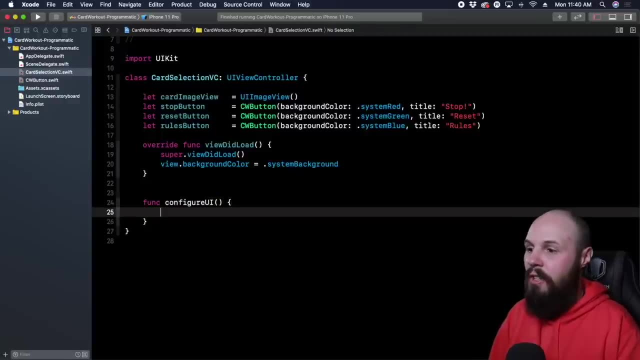 understand what's actually going on. so the first function i'm going to create is kind of like an overall function called func- configure ui. so this is kind of like the overall function that configures our ui and i'm going to make sure we call that in view to load configure ui. there's nothing. 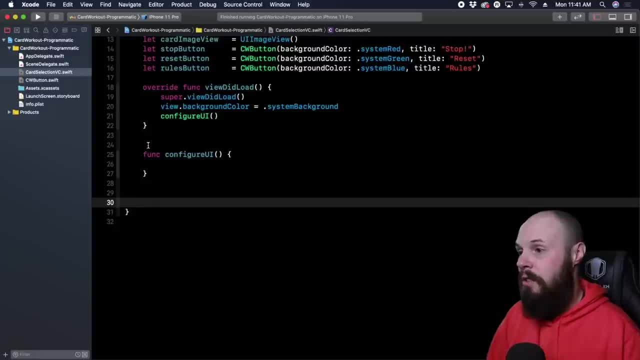 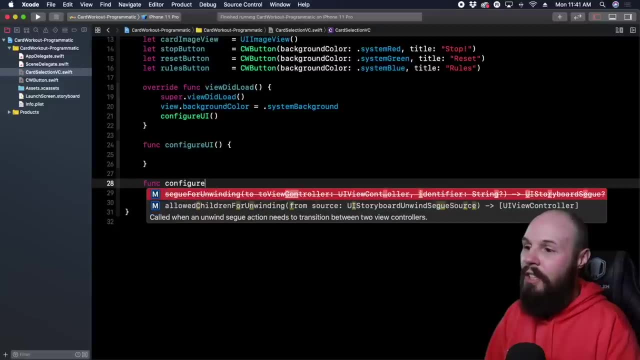 in it yet we're about to fix that. so down here and then another function, you know. let me go back to one space. in between, i keep forgetting that my- uh, my screen resolution is so big, so we'll do func, configure card image view. okay, so now we're going to do this stuff specific to our card image view. 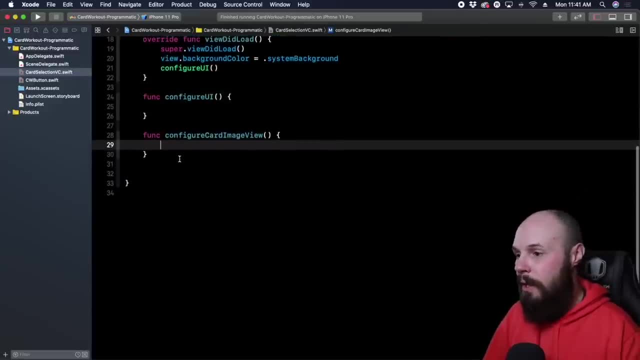 again. like i said, i'm breaking this out step by step. so the card image view. the first thing you want to do- and you're going to forget this, i guarantee you- when you're doing programmatic ui, um, you have to add the sub view to the view. so we do view. 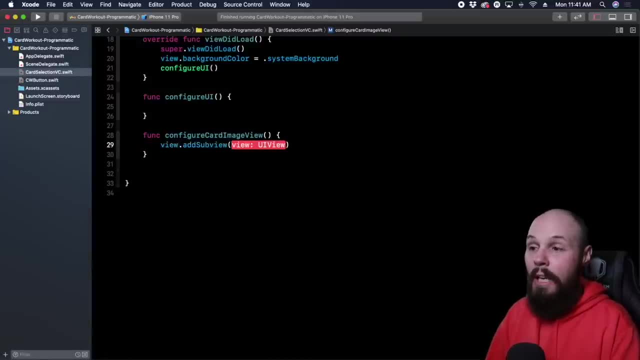 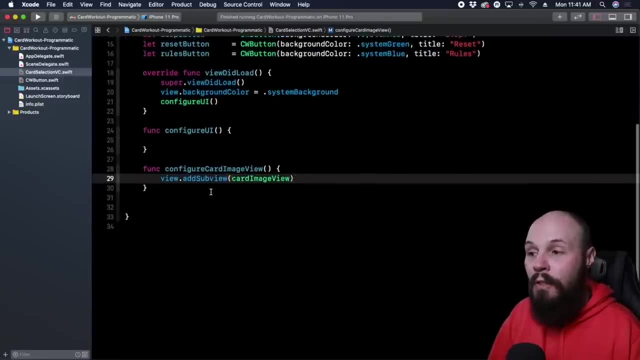 me. i'll explain that more in a second viewadd sub view. and then the view we want to add is our card image view. remember we created that card image view up here on line 13.. so what viewadd sub view is? it is the equivalent of us hitting the plus button searching for an image view. and 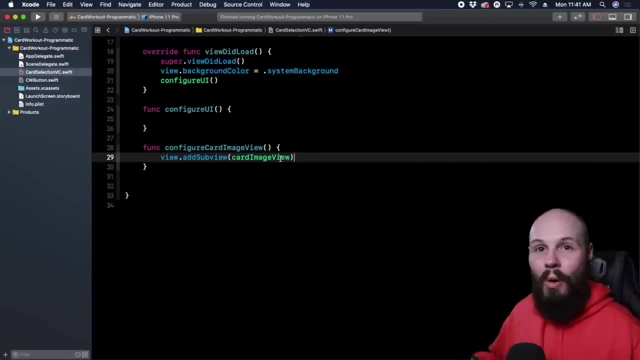 dragging it onto the storyboard. when we drag it onto the storyboard, we're adding the sub view to the view. so you're doing that exact same thing in this line of code, just like if you never dragged a ui image view onto the screen. like you can't, you're not going to see it on. 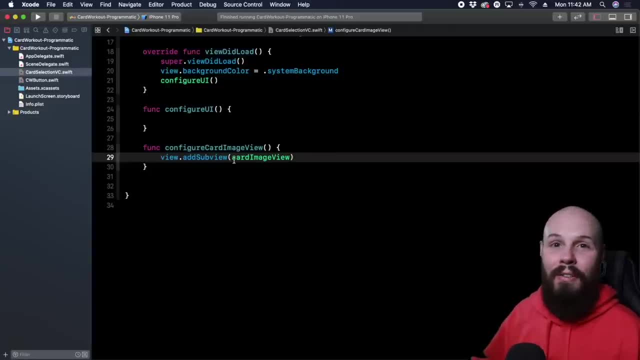 screen. if you don't do viewadd sub view, you're not going to see that view and again, i guarantee you some time throughout your career you're going to forget to add the sub view to the view and you're going to be like: wait, where's my view? why didn't it show up? so hugely important line of code. 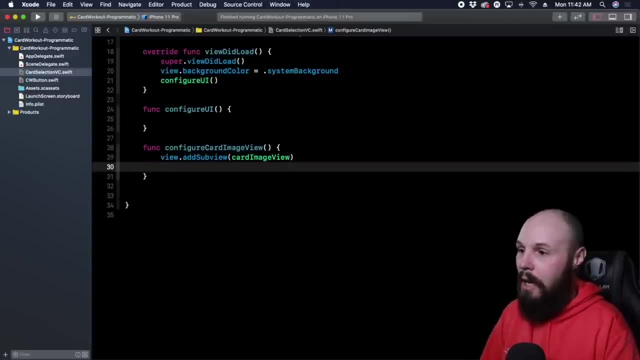 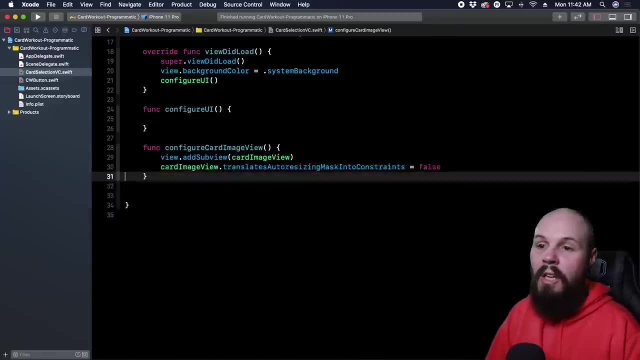 and again, another important line of code when you're doing your constraints is to: uh, card image view, dot. member tamic. translates auto resizing mass into constraints equals false. and again this line basically just says: hey, use auto layout on this object. so next up, before we go into the constraints, is: we want to give the image view an image. so card image view, dot image. 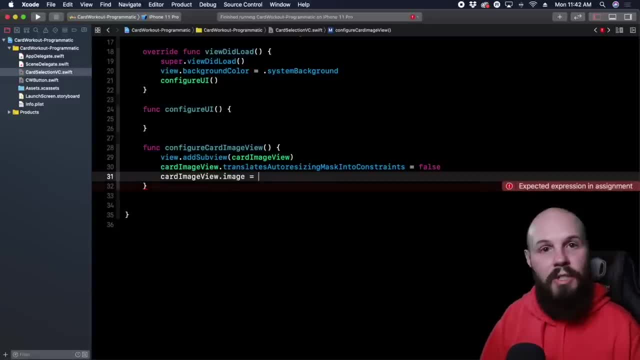 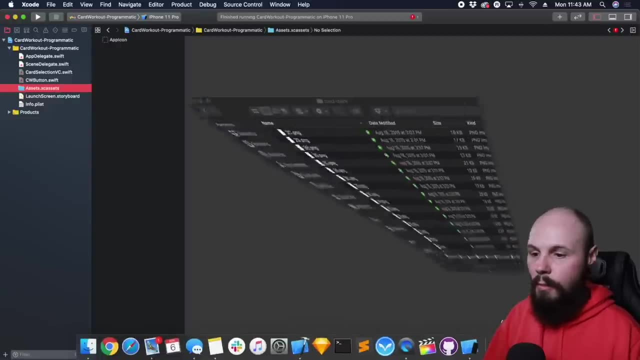 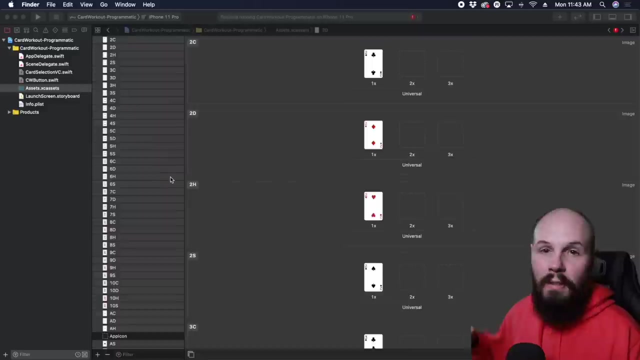 equals. oh wait, a minute. we haven't brought in our assets yet, so let's do that again. same thing we did in the storyboard. we're just going to drag in all of our assets to this assets folder again. i have them down here ready to go, so click on that, drag them in. there we go. all our assets are now. 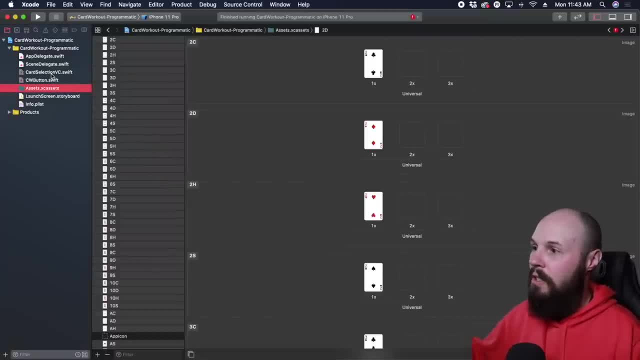 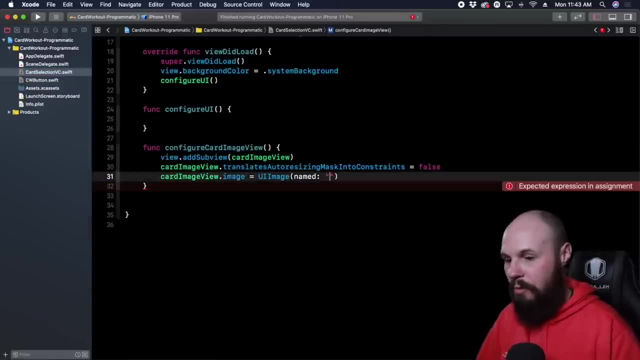 in again same exact thing we did for storyboard. this is repetitive. let's go back to our card selection screen. we can give this a ui image, named, and quotation marks, as that's the ace of spades. so we're going to do it there. uh, for now. so our object exists. um it, it's in the it's in the sub view. uh, we're. 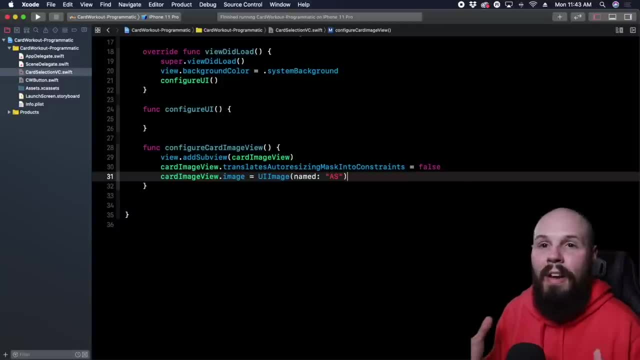 telling it to use auto layout, and we've given it an image. the only thing we haven't done is give it the constraints. remember, it needs to know a width, a height, an x and y coordinate. well, that's what we got to do with the constraints. so, uh, here we go. programmatic constraints. uh, this is the big. 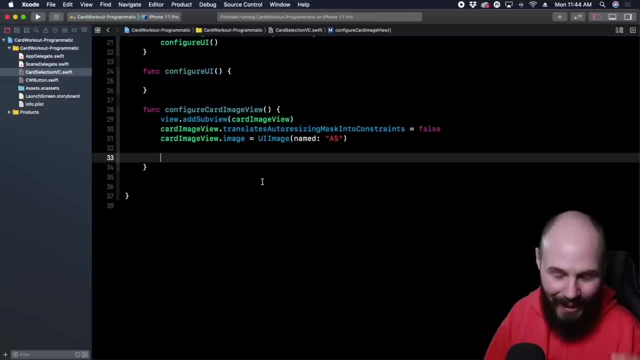 learning lesson of the next few videos. lucky for you, we're going to get a ton of practice at it. uh, you're even going to think, hey, this is really, really repetitive. um, but hey, we're going to drill the point home. so ns, layout constraint is what you type. and now remember, i said a rule of thumb is: 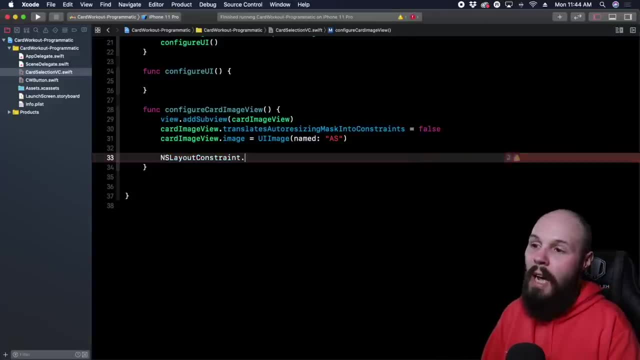 four constraints per object. so if you do ns layout constraint dot activate, you see it takes in an array of constraints. this is where we're going to put in our four constraints. so do open and close brackets for the array. now i'm going to hit return in between. 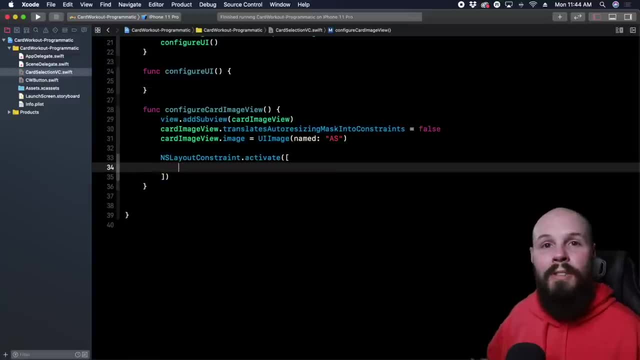 because i want to do this line by line, as you'll see. so what we're about to do now is the same thing we did when we hit the little tie fighter at the bottom and pinned it to the edges and set height and width. right same exact thing, except in code. so the first thing we want: 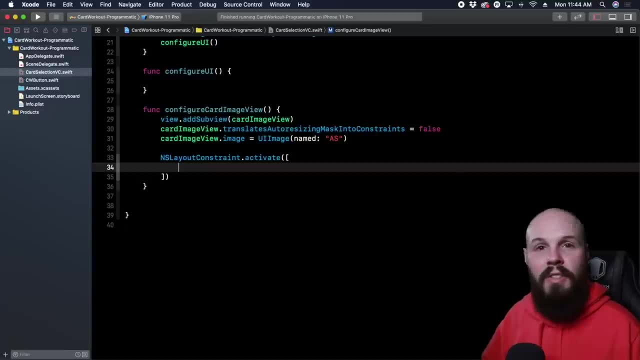 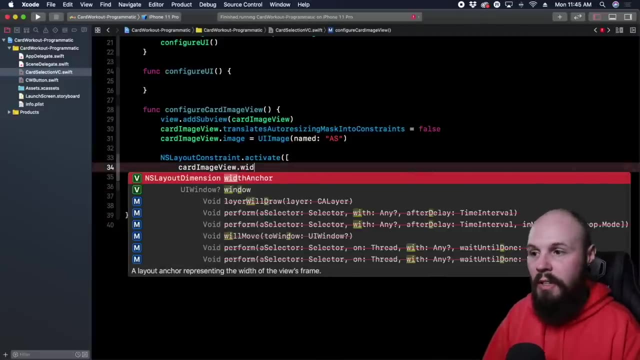 to do on our card is set the width and height. remember we did 250 by 350. so you do card image view dot width, anchor. so anchors are the big thing that you're going to be using. so with anchor dot constraint, remember we're setting the constraints and you see, you get a lot of options. 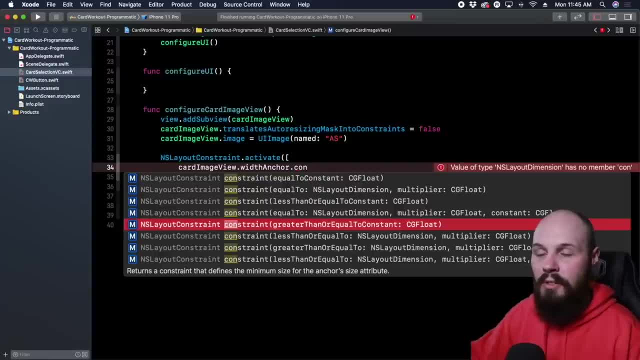 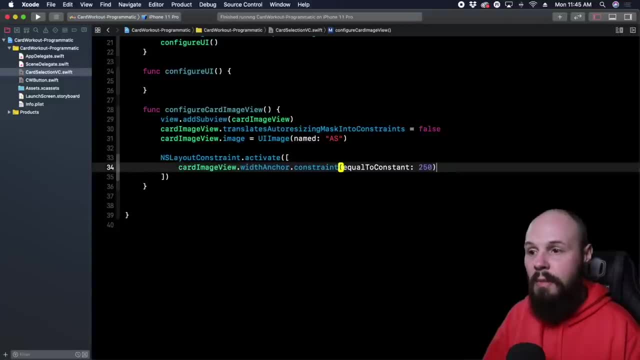 remember, because i said you can do constraints so many different ways. well, here are all the options. we're obviously going to keep it simple. so the constraint is going to be equal to constant. so the constant we gave it, remember, was 250. that's the width, i think. same thing for the 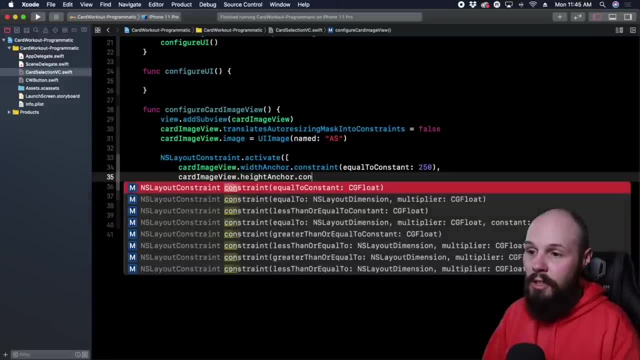 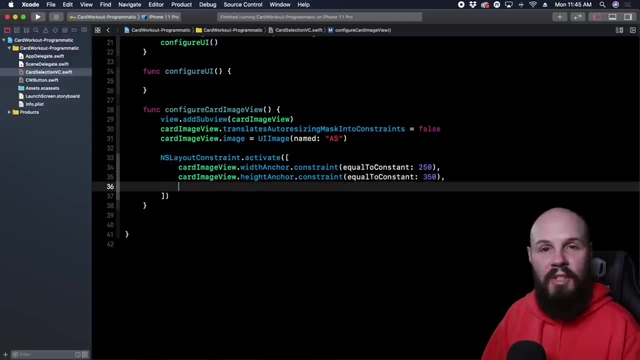 height. card image view dot. height: anchor dot constraint equals 350.. so again same exact thing we did in storyboard, just in code. now we wanted to remember: center it horizontally in the container, so you do. card image view- dot center x anchor right. center it horizontally in the container, so you do. 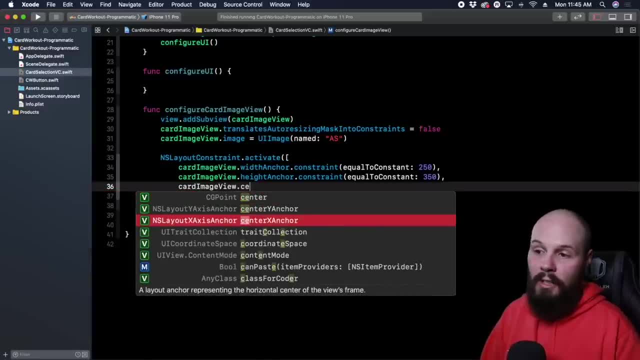 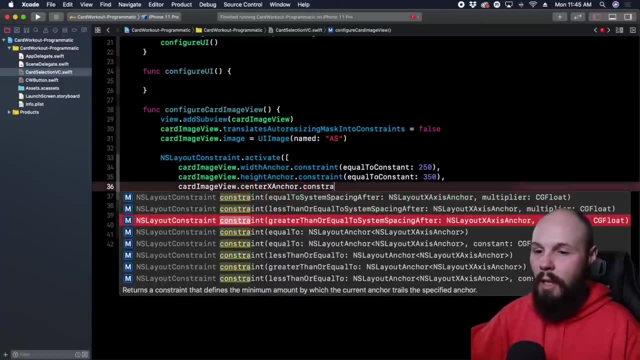 card image view: dot center x- anchor. right center x- anchor. so you do. card image view: dot center x- anchor centered on the x-axis dot. constraint equals- and sometimes the order of this gets messed up, um, so you may have to like scroll down for the one you're looking for. uh, constraint equal to, and we. 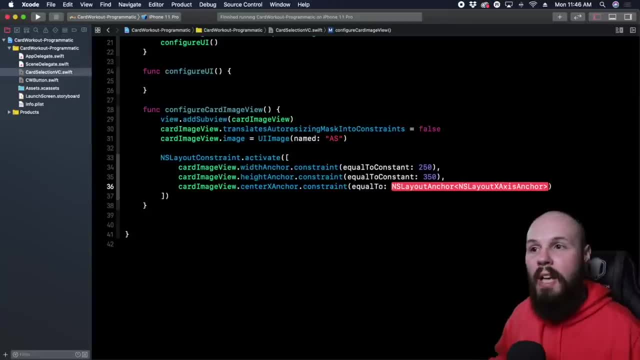 want to make this not equal to a constant right. we're not putting a number in there. remember we said the views center right. so we want to do view dot center x anchor. so what this is saying is remember how i said: every view controller, uh, comes with a view that covers up the whole screen, that's. 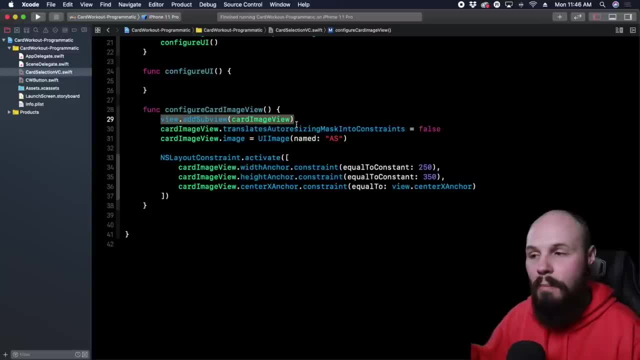 what we're doing here- view dot, add sub view, writing it to that view controller's main view. so what we're doing here is we're centering the card image view exactly with the views center x anchor, so basically center it in the view, just like we did again with the constraints on storyboard. 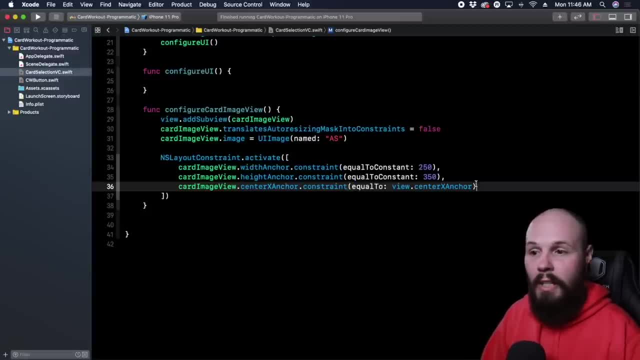 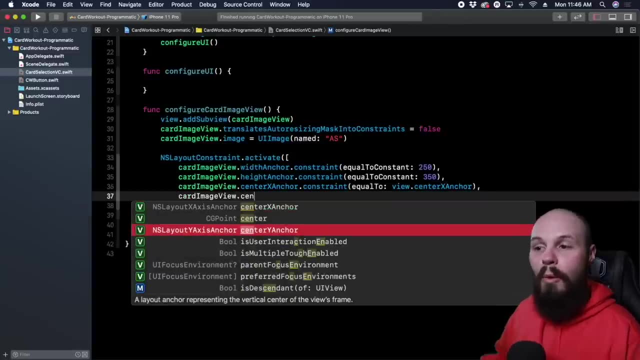 now the last thing we need again right x coordinate, y coordinate, height width. well, we have height width and x, now we just need the y. so card image view, dot center, y anchor. remember we centered this card image view and then moved it up 75 points. well, that's what we're going to do here, dot. 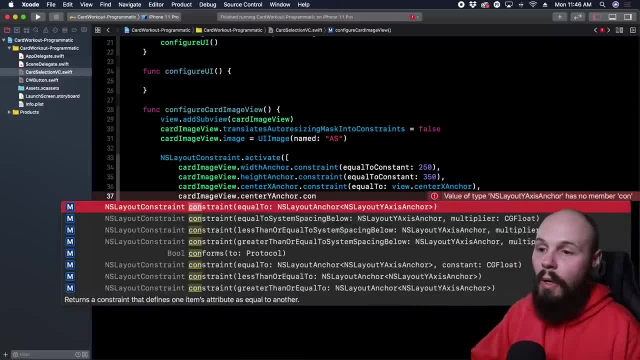 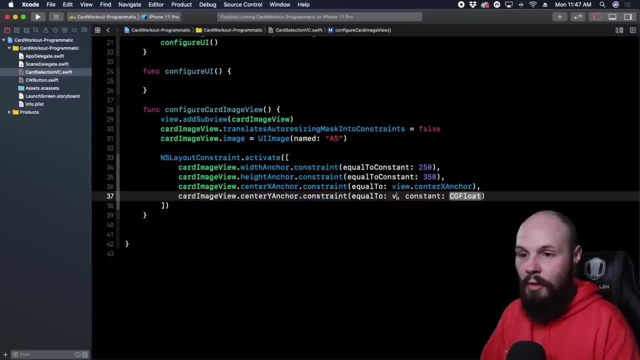 constraint dot now not just equal to an anchor, we want to have it equal to an anchor with a constant. again it's down here, so you'll see- equal to the anchor which is going to be the view dot center y anchor, and then the constant- remember this is how we moved it back up- is negative 75. that's how we. 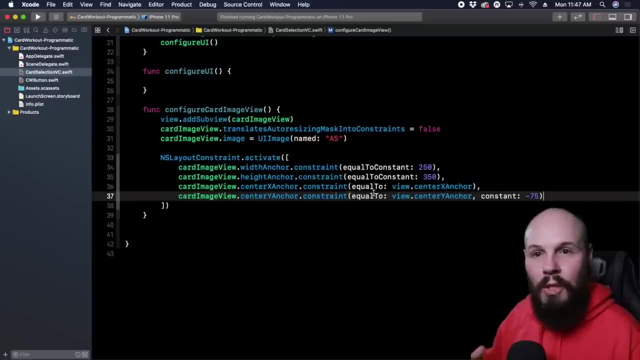 slid it up. so if that was a little bit confusing, don't worry, we're going to do that like 15 more times. so maybe not 15, a lot more times. so you're going to get plenty of practice at it. definitely feel free to rewind the video and watch that again, but just know that we're going to be doing. 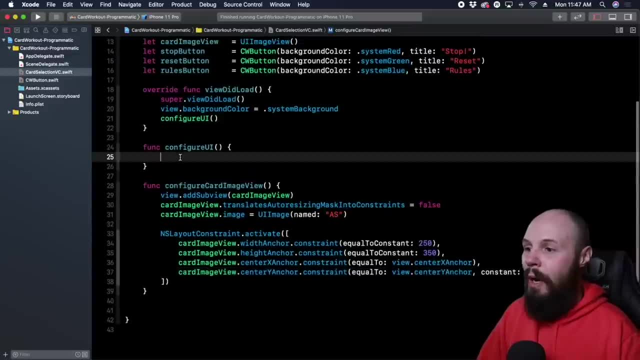 this a lot over the next couple videos. so now here in configure ui, let's call configure card image view and then configure ui gets called and view did load. so when i run this we should see our card placed. uh, where it's placed when we did it before and here we are, there's our card. am i in dark? 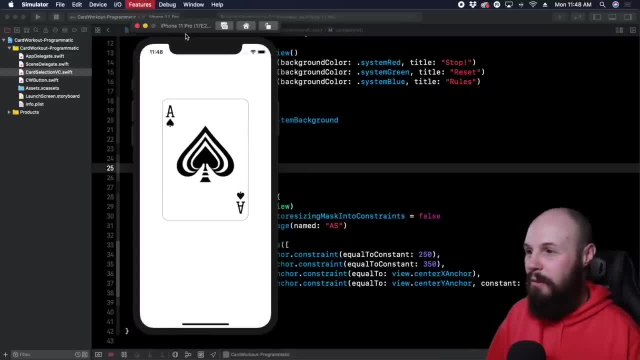 mode. command shift a. okay, i must have been like left over in dark mode from the previous run. okay, i thought i messed something up. so, okay, if that happens, do command shift a to go back to light mode. but anyway, there's our card, Exactly where we laid it out when we did it in storyboard, except let me stop this, you see. 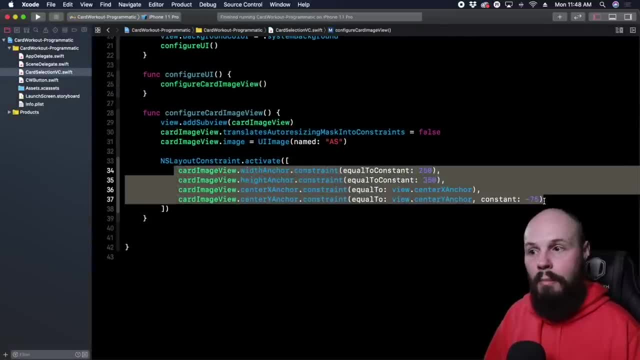 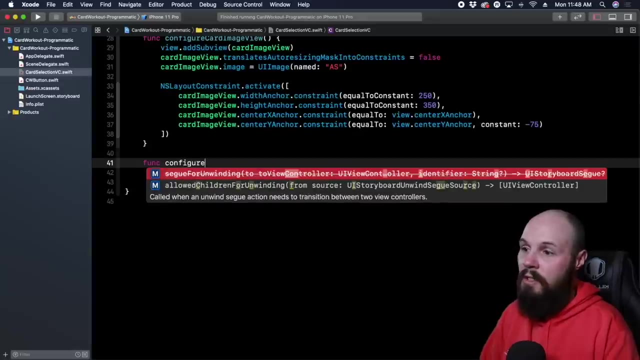 These four lines of code is the equivalent to, you know, Setting the height, setting the width, pinning it to the center right, all that stuff We did, you know, from the tie fighter button. you just do it in code right here. same thing. now We configure the rest of our elements. so the next function will slide up a little bit funk: configure, stop button. 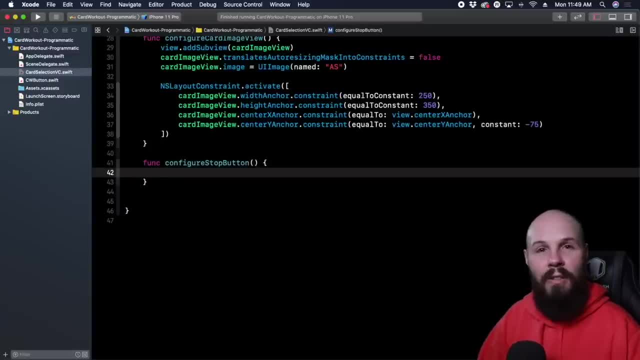 See here and you'll start to see why doing it programmatically adds a lot of you know code to your view controllers. That was just done on storyboard, so again back to the pros and cons. Anyway, what's the first thing you need to do in doing programmatic view dot add, sub view, stop button again. 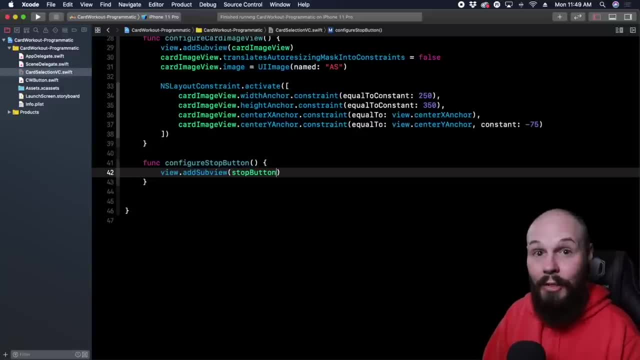 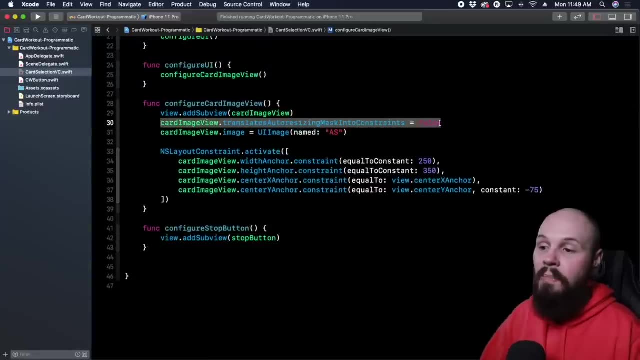 This is the equivalent of dragging the button onto the storyboard. right, you have to do that before you can do anything. Now, what we don't have to do- remember in the card image view we did- translates auto resizing mask into constraints. We don't have to type that line of code here. Why, if you remember, back in CW button. 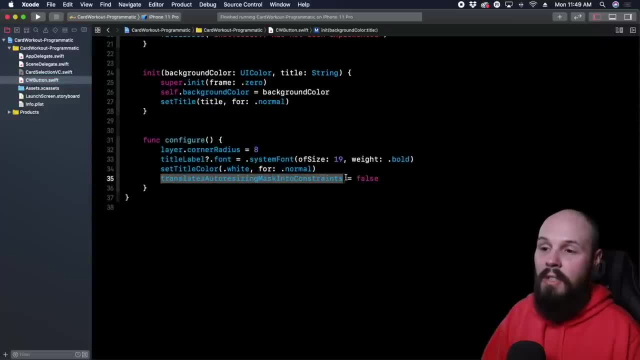 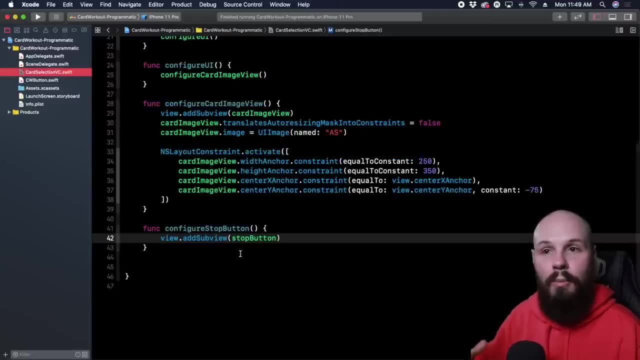 We included that line in our configure. translates auto resizing mass into constraints. So every CW button is already going to have this set the false, so that way we don't have to write this code again. That's a way to be dry, right, don't repeat yourself. another benefit of creating: 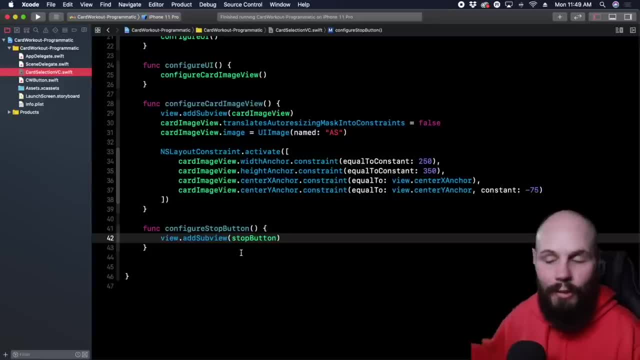 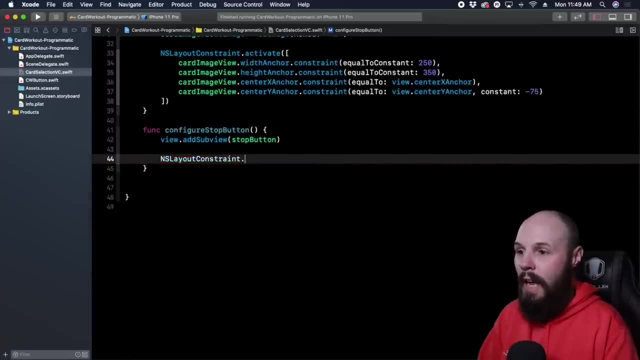 You know a subclass. all that code lives in CW button. We don't have to retype it. So all that leaves for us, at least for now, is setting the constraints. so again, NS layout constraint, dot activate, and this takes an array of Constraints, very similar, right. like I said, this is going to get repetitive, but again, repetition is key. so you do, stop button. 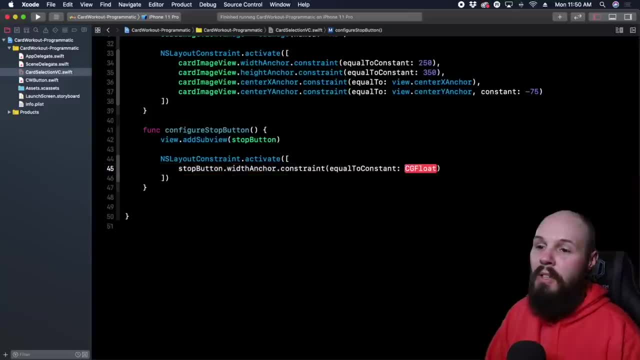 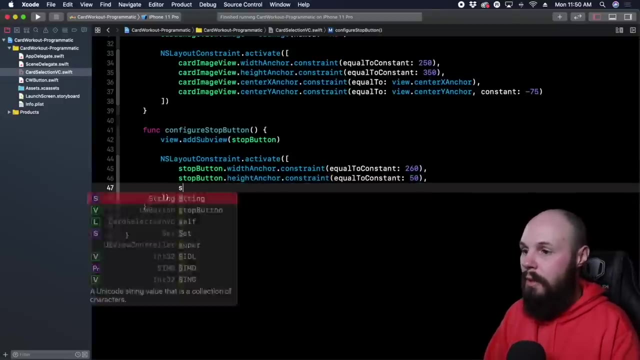 Dot width anchor. remember, we set the constraint, we set the width equal to 260, Same thing we did in storyboard- and we set the height to 50. so let's do that to stop button dot. height anchor Constraint equals 50. cool, cool, cool. now What else did we do? right, We centered it on the x-axis. so stop button dot. 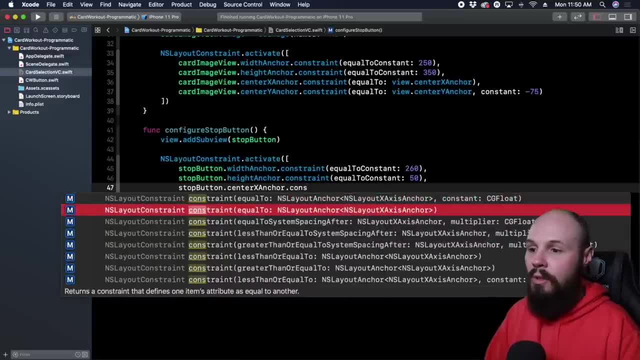 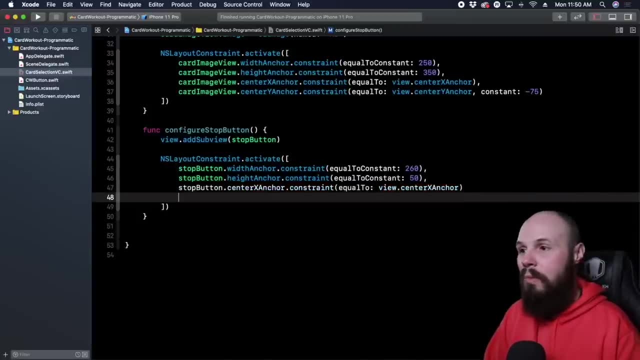 Center X anchor constraint. it's equal to: again We want to pass in the layout anchor View: dot Center X anchor. and then now we need a y-axis. well, We pinned it to the bottom of the card image view. now This is a key point when doing your layout programmatically. is that the order matters, right like? let me type this out: 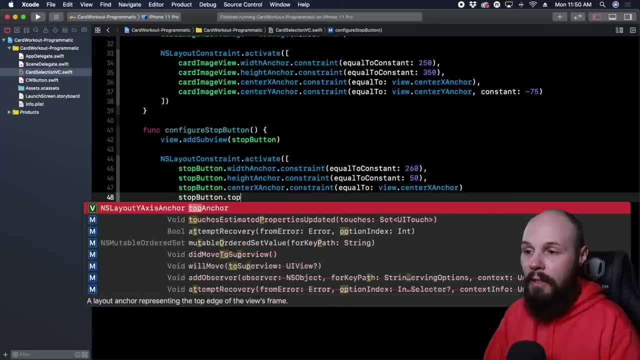 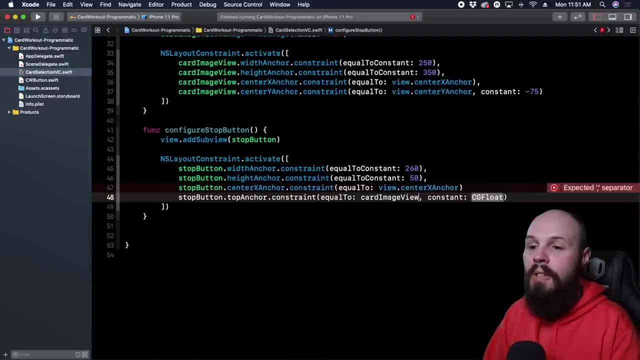 And then explain that. so stop button- dot top anchor. So the top of the stop button we want to pin to again passing the anchor and a constant, We want to pin it to card image view: dot bottom Anchor. so we're pinning it to the bottom of the card image view and think about we did like 30. 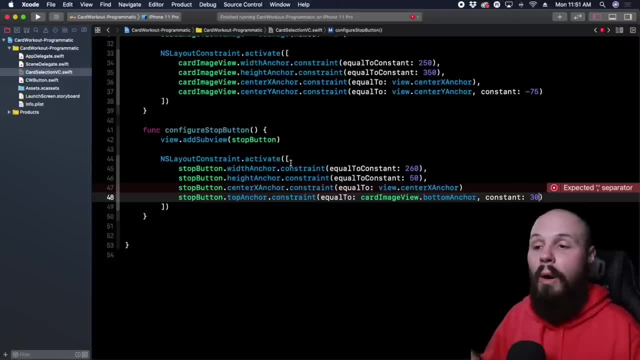 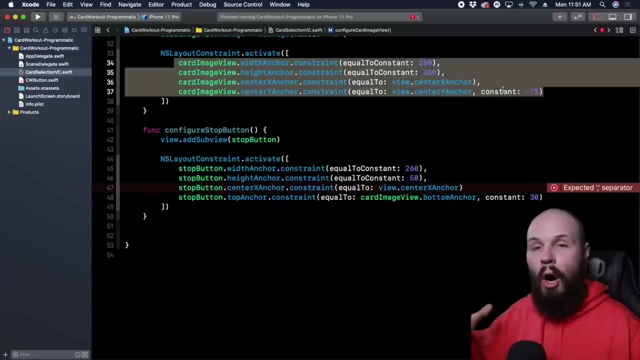 It's irrelevant. so anyway, the thing I wanted to point out was the order Matters right. I can't pin anything to the bottom of the card image view until the card image view is laid out right, because if the Card image view doesn't know where it's at on the screen, 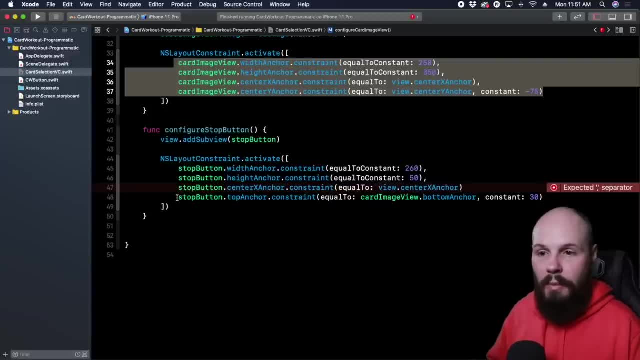 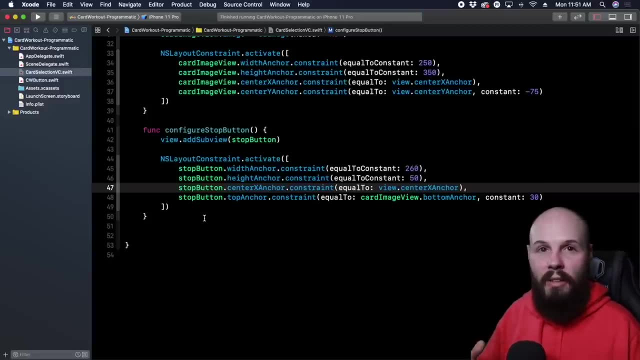 I can't pin the stop button to the bottom of it. that looks like I'm getting yelled X. I don't have comma there. so anyway, the order in which you lay it out matters. And if you remember, when we laid this out via storyboard I said, like we did, the card image view first, because that was kind of like our, our anchor of our UI. we were going: 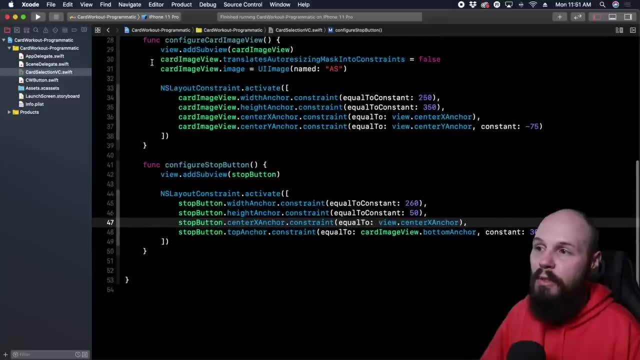 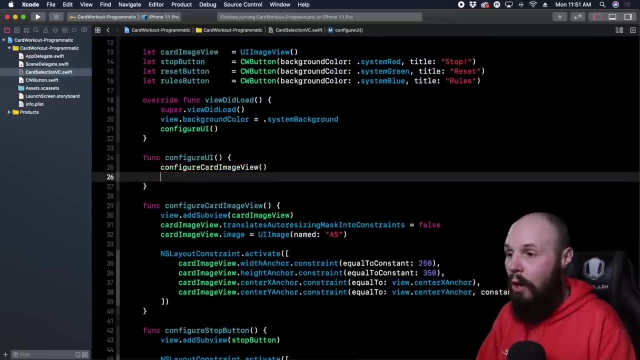 To be pinning everything else to that. so again, That's why we configured the card image view first, and then the stop button, and where the order comes in To play, you can see we're gonna call configure card image view and then we're gonna call configure stop button. 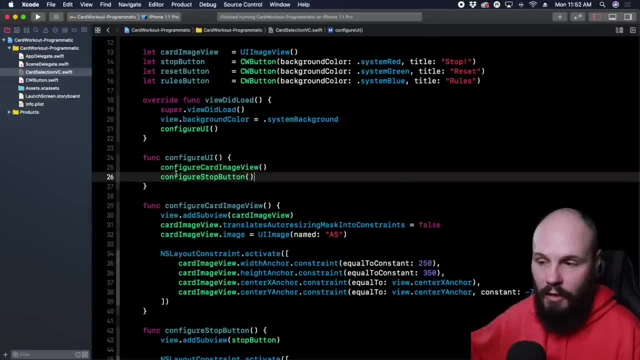 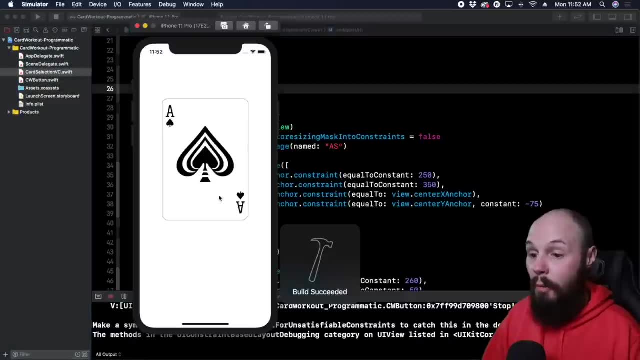 So right, so the card image you gets configured and then the stop button gets configured, so that ensures the order that we're looking at Here. so, now that we've called it, Let's run this and we should see our stop button on our app. We don't crash, crash, We're not a crash, but some constraints are messed up. so 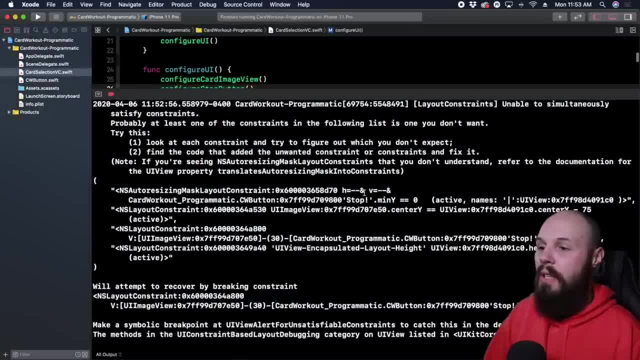 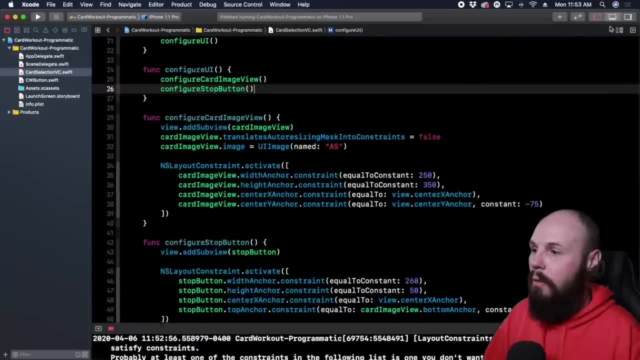 Let's see here. Okay, so usually when you see all this right, this means you forgot to set auto resizing mask equals the false Tamek, right? Let's get rid of this. but remember, I did this in the CW button, right? oh man, translates auto resizing mask constraints into false. 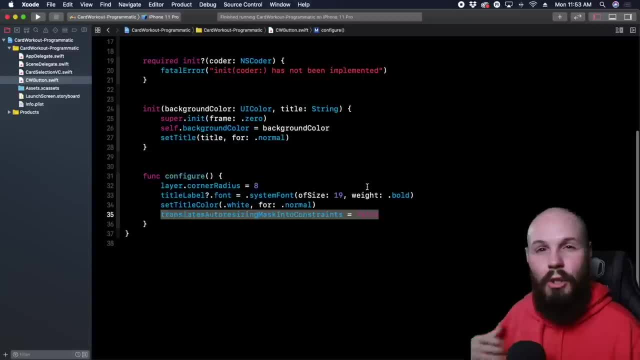 But what I forgot to do in the last video, and again, just to show you how easily bugs can come up. I like to keep these mistakes in there, So you don't think you have to be perfect as a programmer. trust me, ask any programmer that's been doing this long. 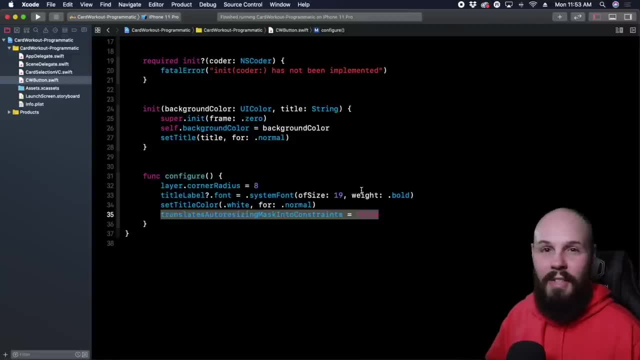 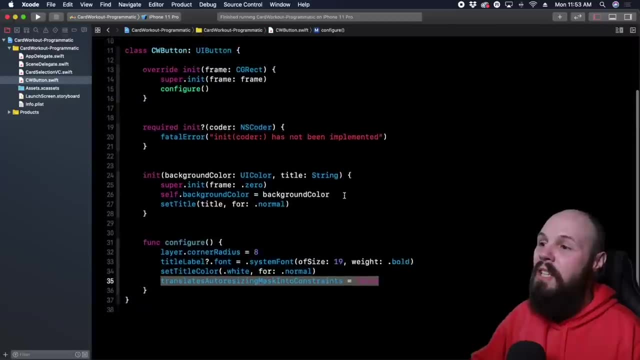 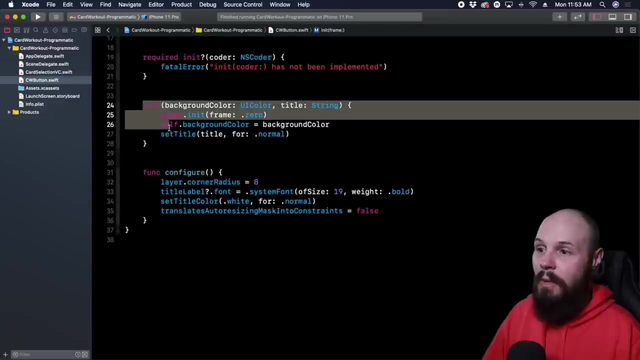 They make silly mistakes non-stop, all day, every day. They say programming sometimes will make you feel like the smartest person alive and then also like the dumbest person alive. So the mistake I made was super simple, right? remember, in this initial Initializer, right, our default one I called configure method. well, in this custom initializer method, look. 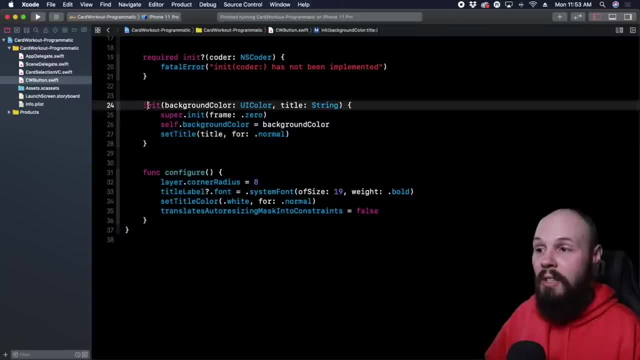 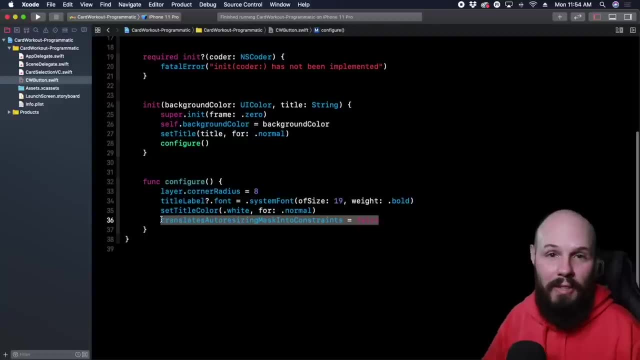 I forgot to call configure. so it did call this initializer But it didn't call the configure method to do all of our other stuff here, which includes Translates auto resizing mask into constraints. so now by calling configure in this initializer- and remember we're using this initializer up here- 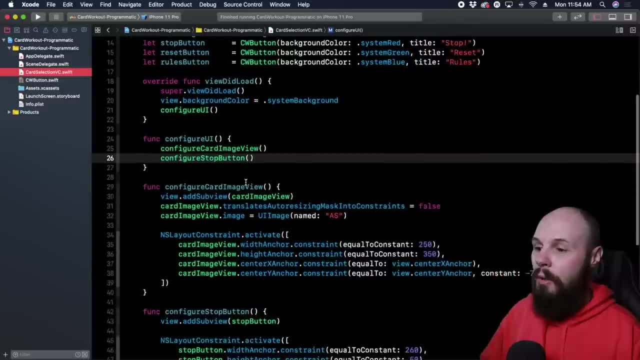 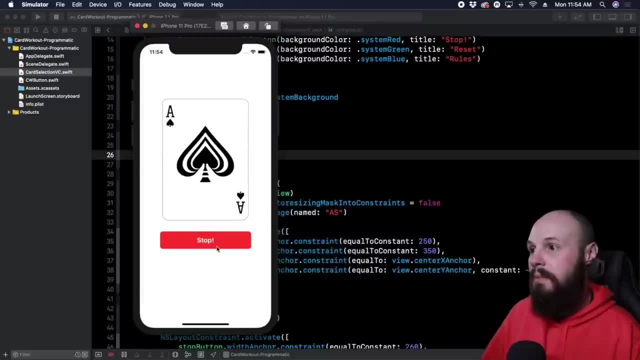 Configure was never getting called is basically what I'm trying to say here. so now, when we run it, it will call Configure. we're going to translate the auto resizing mask into constraints and, as you can see, there's our stop button. So let's keep it moving. keep going on with the rest of the buttons here, so do. 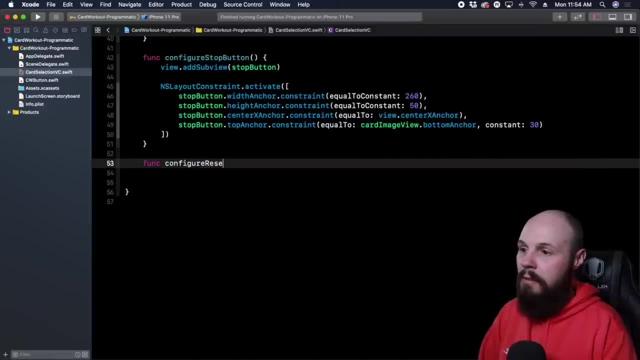 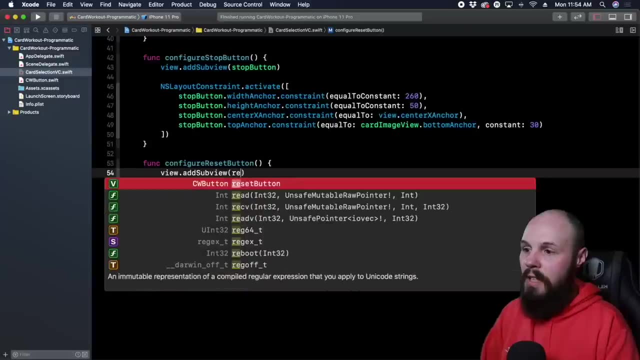 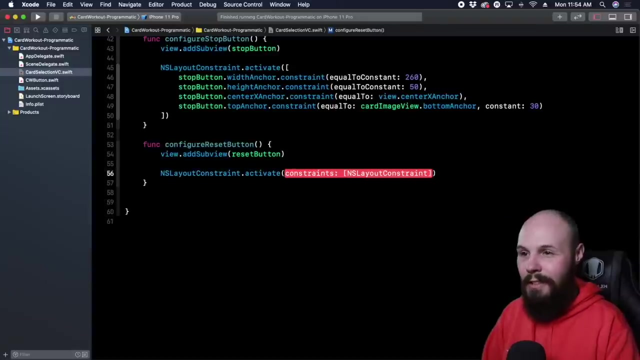 funk, configure, reset button and Very similar stuff. rip. most important thing, view dot, add sub view, reset button. and Now we need to lay out the constraints. so NS layout constraint- again repetitive. but You're going to get practice right and that's good. You're going to be good at it. 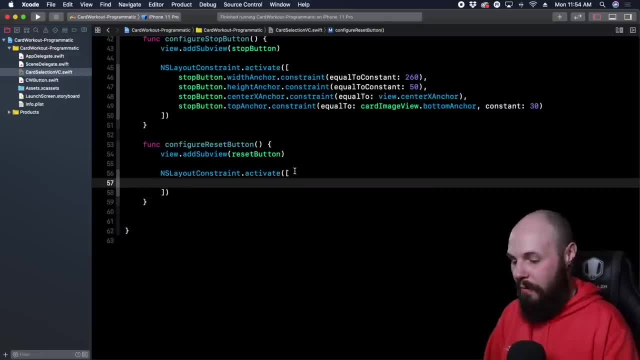 Passing the array, go down to the next line, and here we go. so now we do reset button dot. right, We have the width, so with anchor that Constraint- remember it was 115- and then we also had the height, which was 50. so reset button dot height, anchor that constraint. 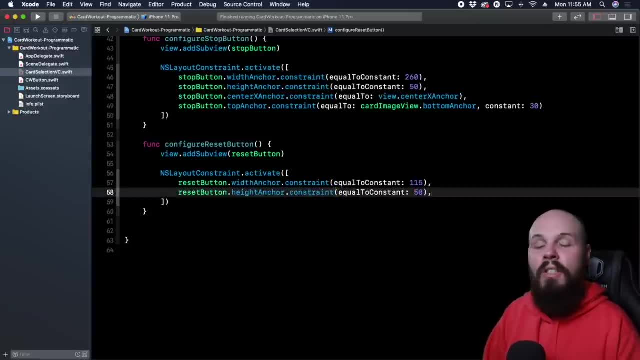 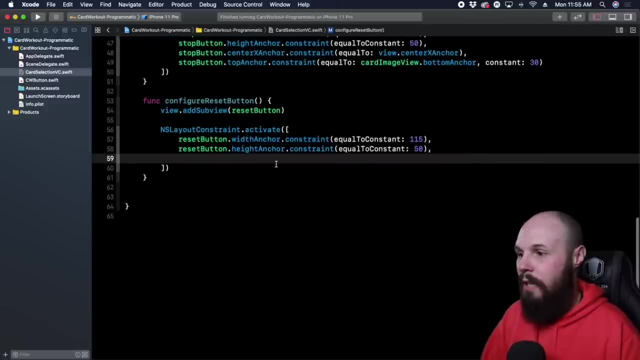 Equals 50, so we had the width and height. now these constraints get a little different. if you remember, we pinned the left side of the reset button to the leading anchor of The stop button, so I'll show you how to do that. so reset button dot leading anchor, remember leading. 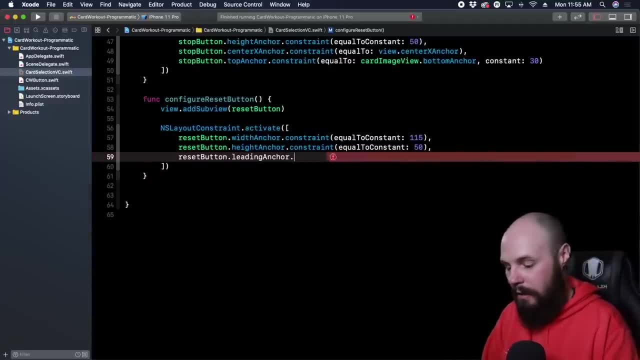 I was on the left. again, in a left to right language dot constraint equals Stop button right. we want to pin it to the stop buttons dot leading anchor. so again, This is going to line up the left sides of the button and actually the constant is zero, because so anytime a constant is zero. 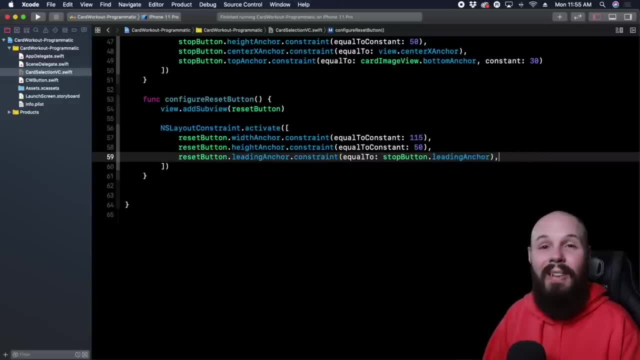 You don't have to have it. I accidentally selected the wrong one. So that's going to line up the left sides of the button, which is exactly what we wanted. now We just need the y coordinate, which again We pinned it to the top, I'm sorry, to the bottom of the stop button. so reset button dot. top anchor dot. constraint is. 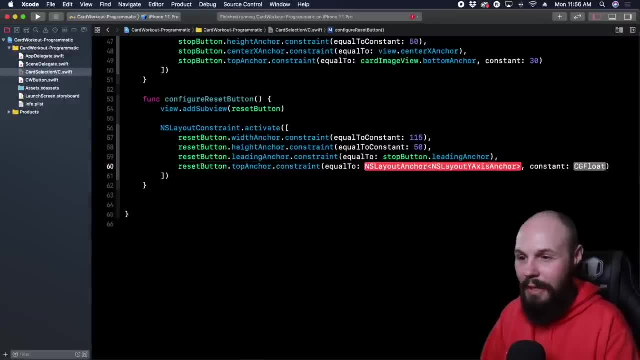 Equal to. again, I hate when these get mixed up, but no, that was actually right at the top. so stop button, dot bottom anchor and In the constant I believe we did 20. So now our reset button is configured again: a width of 115, a height of 50. 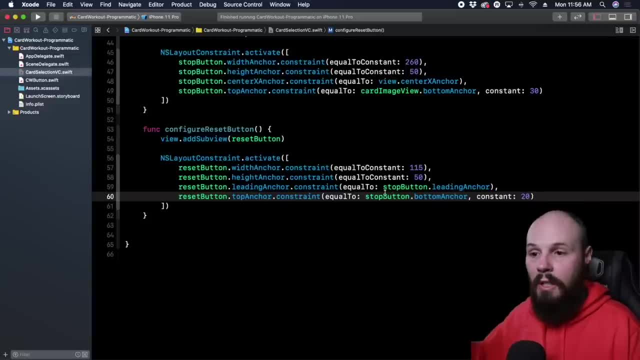 We align the left sides or the leading sides of the to the stop button and then we pinned it to the bottom of the stop button. Now that should all be familiar to exactly what we did in the storyboard, again Just doing it in code. like I said, some people like that storyboard how it's all visual and 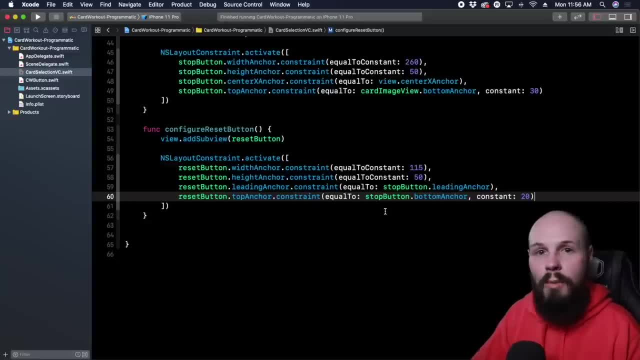 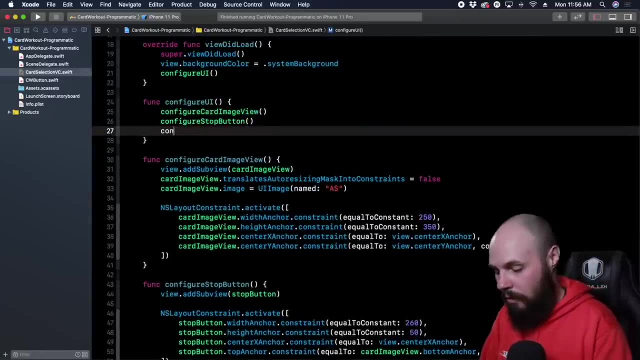 Some people like being able to see the code right in front of them so they can see what's going on without it being kind Of like magically hidden away in the storyboard. Now let's call configure reset button. so configure Reset button. now that's getting called in our configure ui method, which again is getting called and viewed. it load. 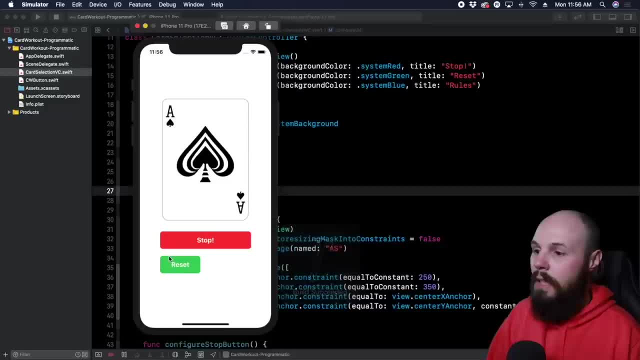 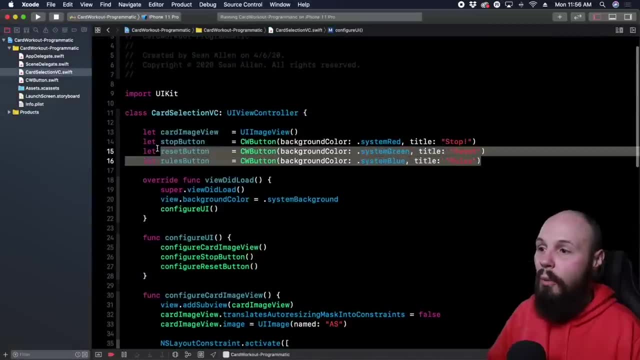 Let's run it and we should see our reset button. there We go, there's reset, So let's stop it. and again, It's all configured with the green and the reset, because we did that up here when we initially created the objects. So the last thing we're going to do is add our rules button and now. 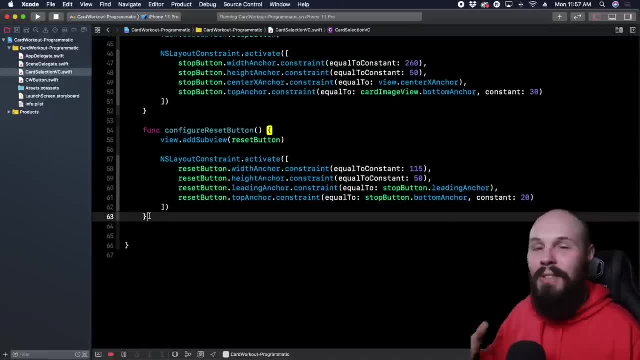 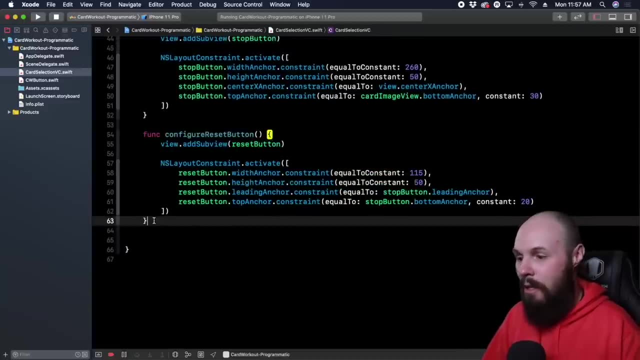 I've been typing these out individually to kind of show you. Oftentimes in the real world I do a lot of copying and pasting when it comes to constraints, because you'll see that's a lot of similar code here. so copy Paste now. copy paste. errors are a thing you're going to make a lot of them. 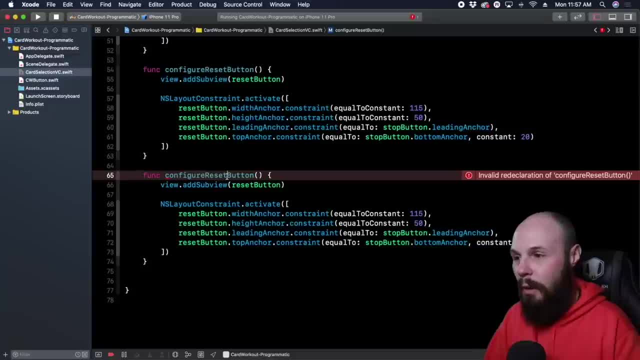 So anytime you copy and paste like this, be very, very careful and double-check. So, instead of configure reset button, We want this to be configure rules button, Cool, and then view dot, add sub. u double click on reset button, Make that rules button and then there is a. there is an edit, all in scope. 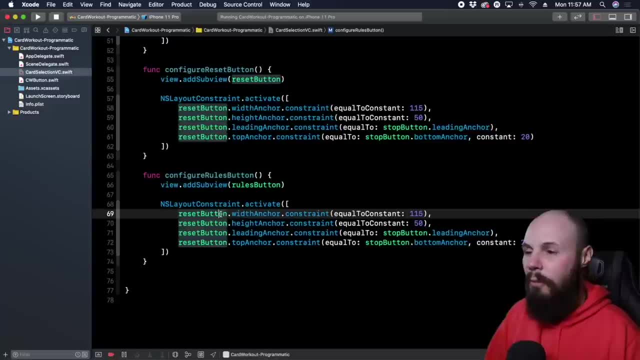 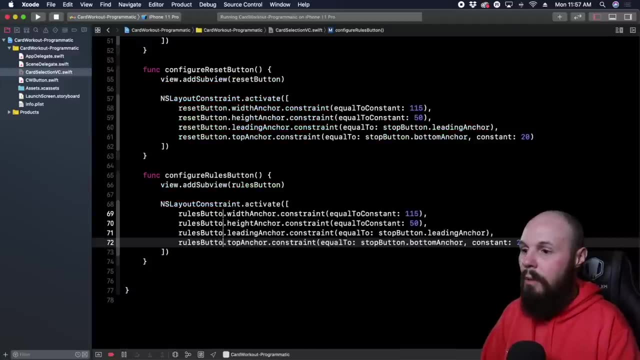 I believe it's like command shift e, I think I don't know. we can look up that shortcut later, But I just prefer it's quicker for me. I hold option, Drag down like that, and just type rules button. There we go. now Let's go line by line here: our width anchor: that is the same, remember. 115 our height. 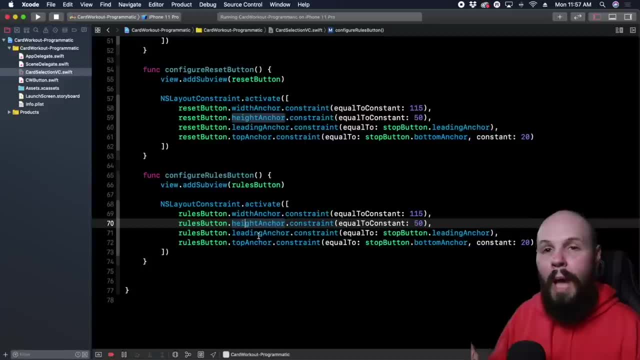 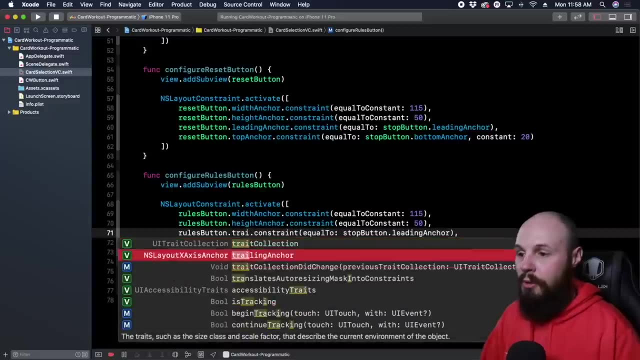 that is the same 50, uh. however, we're not pinning it to the leading of the stop button, we're pinning it to the trailing of the stop button. so double click on leading anchor, change it to trailing anchor and then same thing, equal to stop button dot, trailing anchor. because, remember, we're pinning. 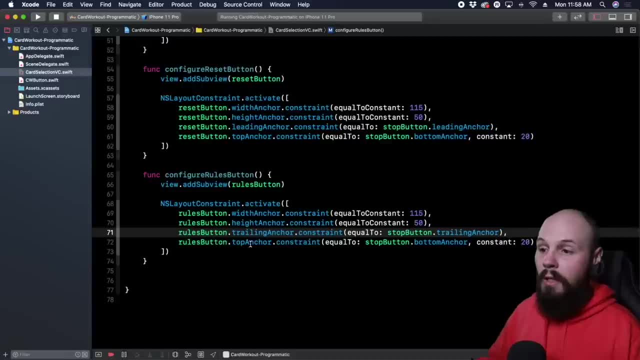 it to the right side of the stop button, now for our rules button, and then rules button, top anchor constraint: same thing, uh. pinning it to the bottom of the stop button at 20- again same thing as the- uh, uh, reset button. so now let's stop this and run it. and we should have. nope, almost, almost had. 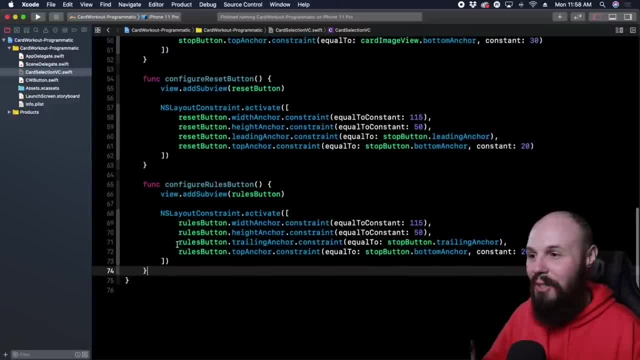 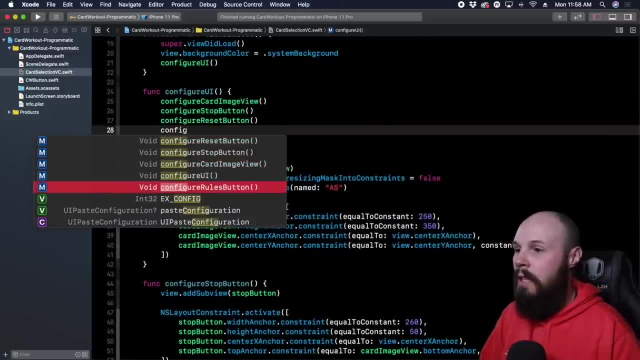 the mistake there. i caught myself, remember. i said you're gonna forget to call your functions all the time, so we got to call configure rules button. so again, configure uh, rules button. and real quick, kind of uh, how i like my functions to read is i compare it to a table of contents- right, like i? 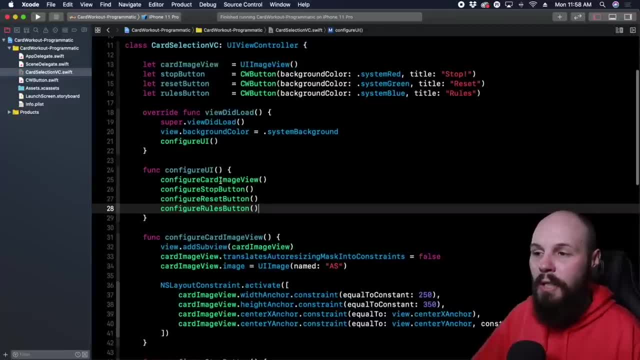 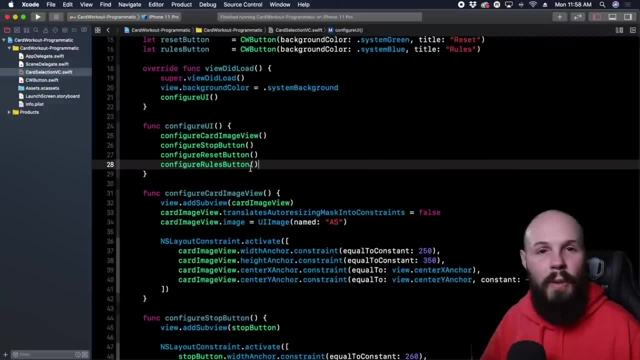 like people, people to come to see: okay, what's configure ui? okay, i'm configuring card image view, i'm configuring the stop button, i'm configuring reset button, i'm configuring rules button, and if that's all they need to know, cool, they can move on to reading the rest of your code. however, if they want to dig in, like, okay, so there must be an issue with. 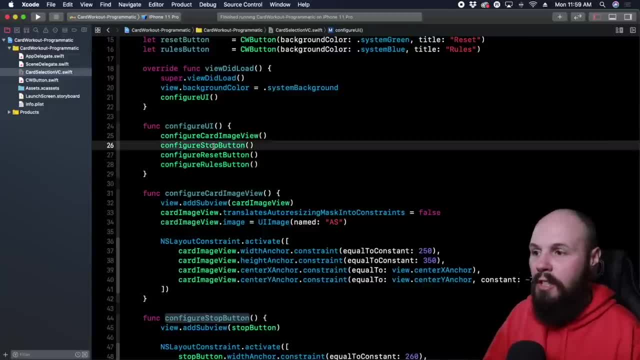 how we're configuring the stop button. cool, i can just dig into the stop button function and how you do that. by the way, if you hold command and click on the function, you'll get a menu here and click jump to definition and it'll it'll. well, it was right there, but if it's in another file, or 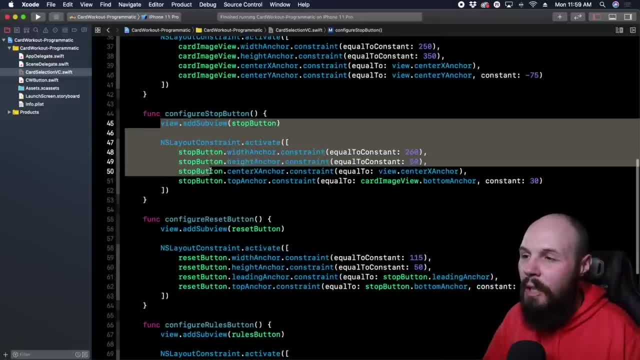 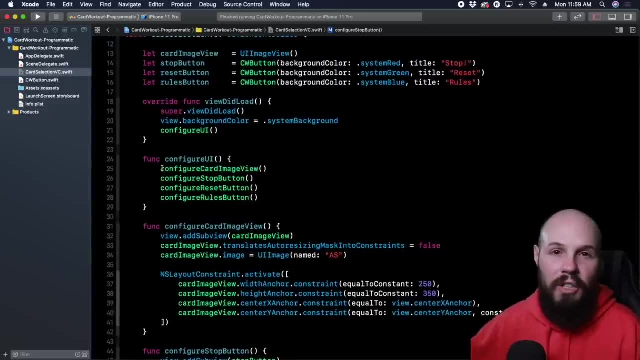 something like that. it'll take you to that file so you can see what's actually going on in configure stop button and you can see what's going on. but again back to the table of contents. you don't want to just have this super long, huge function because that's really hard to read. give them like the list. 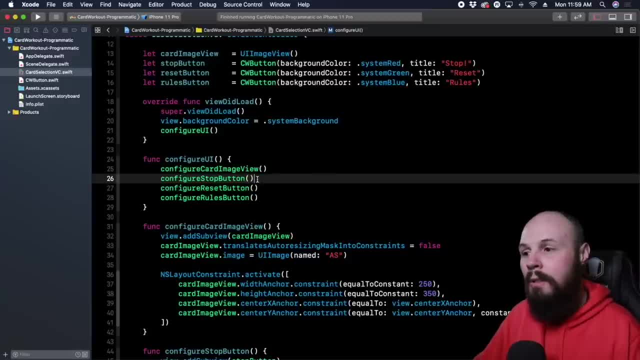 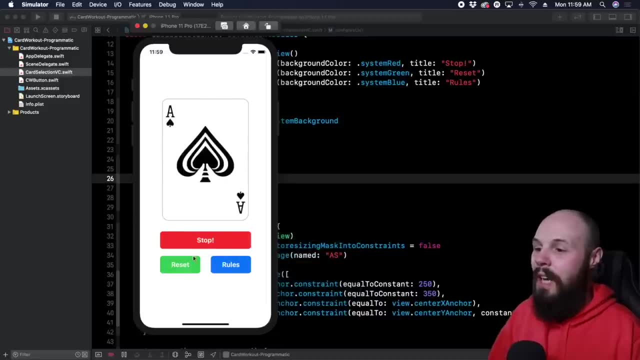 of commands that are going on, and if the reader of the code wants to dig deeper now they can by going into each function. all right, rant over, let's run this and see what we got. we should be done here with this video. yep, there it is. stop reset rules. our ui is laid out programmatically. good to. 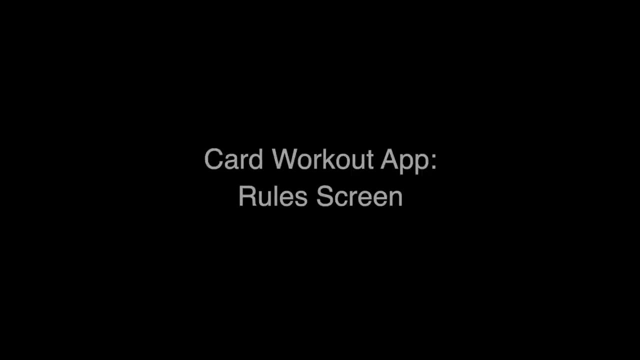 go again, picking right up where we left off. from the last video, you can see that the ui is laid out programmatically. good to go again. picking right up where we left off. from the last video, you can see that the ui is laid out programmatically. good to go. 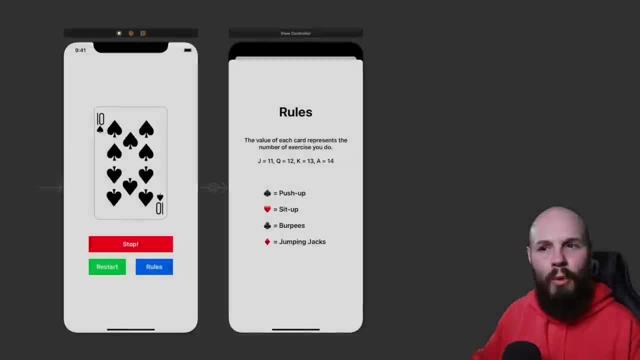 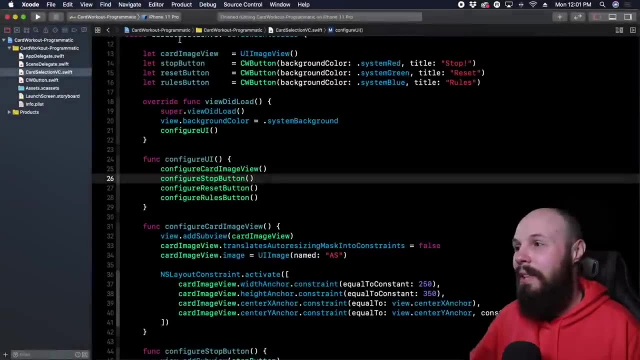 in this video we're going to create our rule screen and remember on storyboard, like we didn't have to do any code at all. we could just configure it all on storyboard. well, that's not quite the case here. uh, let's start building that. uh, click on your card workout folder again. command n: 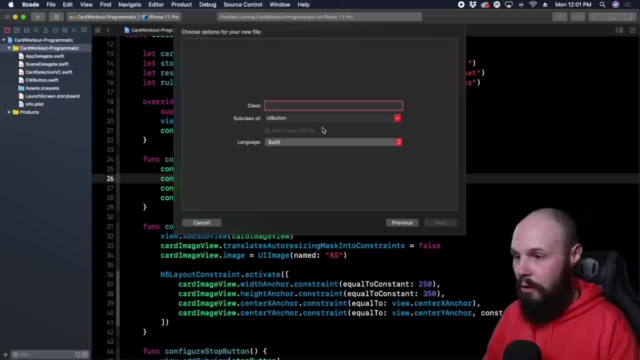 uh, coco touch class. we need to create the view controller, so let's call this the rules uh vc for rules view controller. now, remember it's not a subclass of ui button. make sure you check that. i've done that a thousand times where i forgot to do that and uh created the wrong thing. 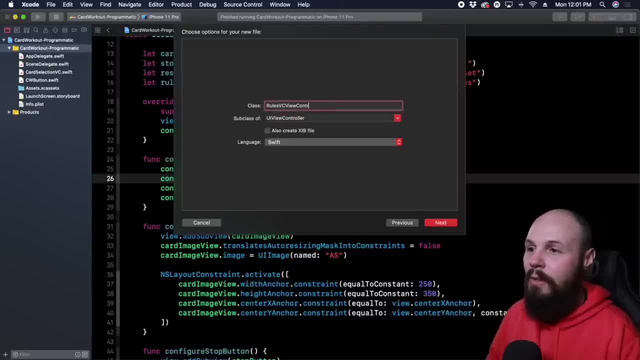 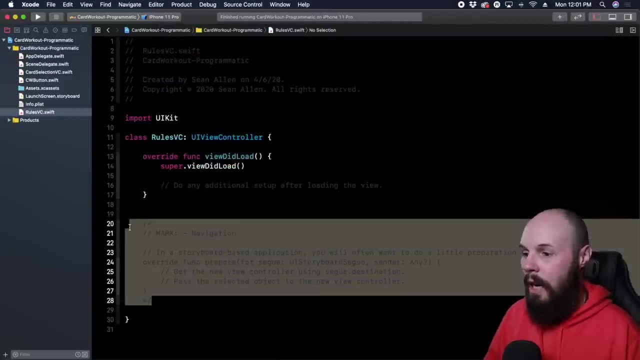 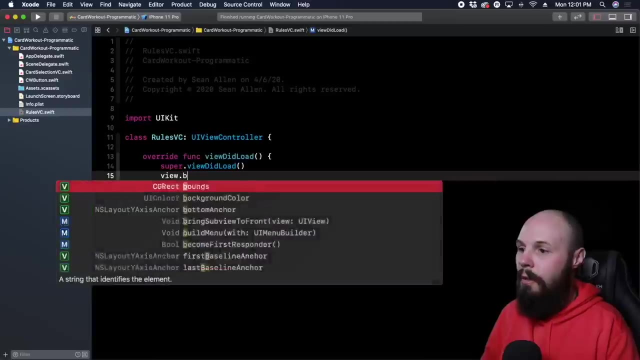 ui view controller and it i hate that it does that it adds view controller to the end of it. nope, we just want rules vc. hit next, uh hit create. cool, here's our empty uh rules vc, and let's not forget to give it a background color: uh background, view dot background. 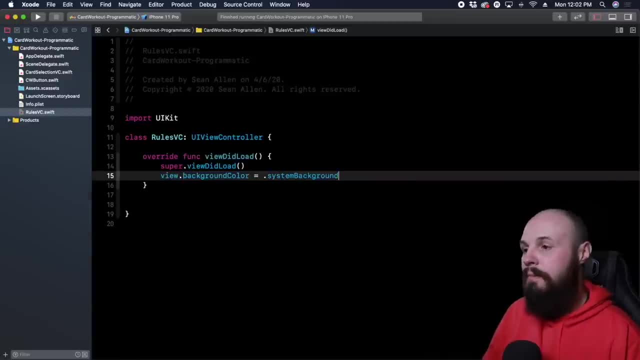 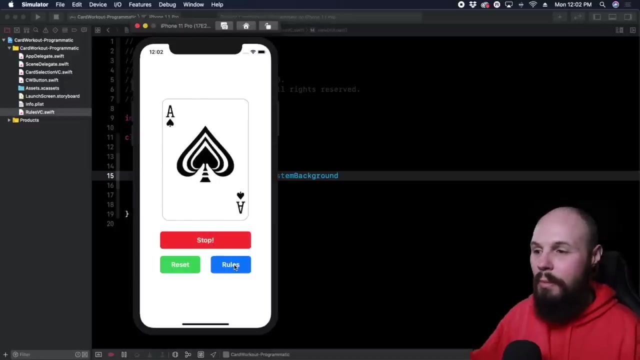 color equals dot system background. there we go, and again the system background: light and light mode, black and dark mode. now, in order to see this screen right when we run our app: um right, let's do this. we run the app. uh okay, rules. uh well, well, remember, we created a segue in the storyboard. uh well, we can't do that in code. segways: the. 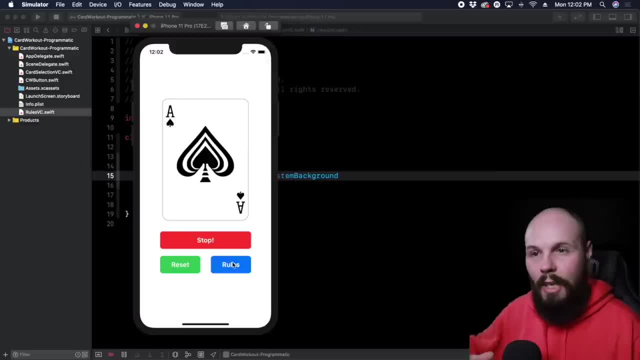 concept of a segue doesn't exist when you do everything in code, like segways are only for interface builder storyboard, um, you can still obviously transition to screens, but they're not called segways, okay. so the concept of a segue is only in storyboard, does not exist when you do it. 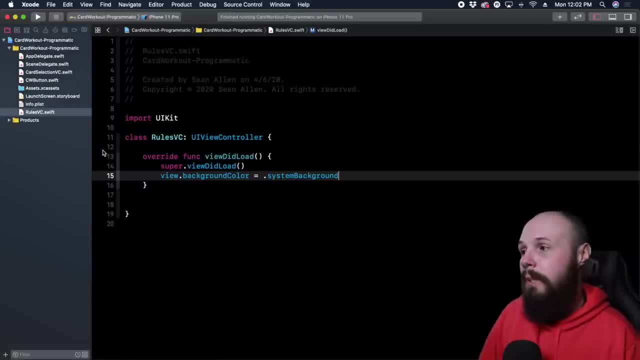 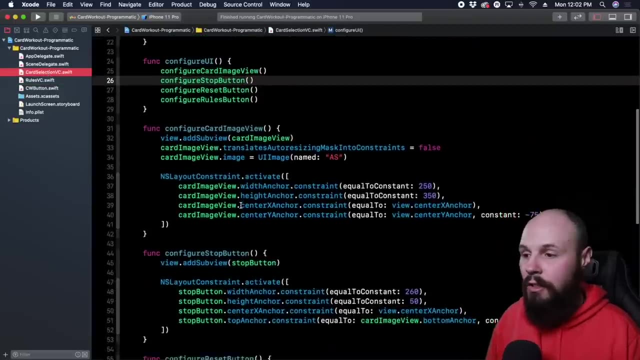 in code. so hit stop. uh, so we need to transition to that screen. so let's actually move this up before i forget and hit card selection vc. now we need to add an action to our rules button. so scroll down to your rules button. uh, the way we can add an action like what? 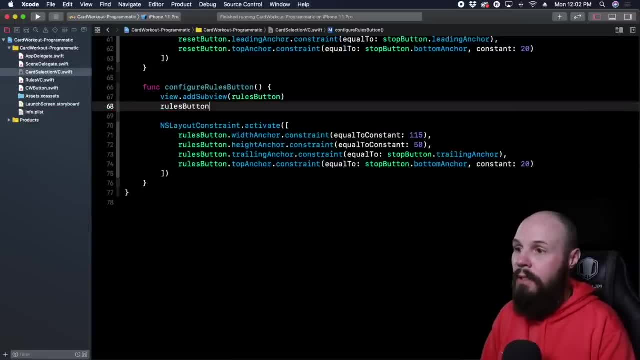 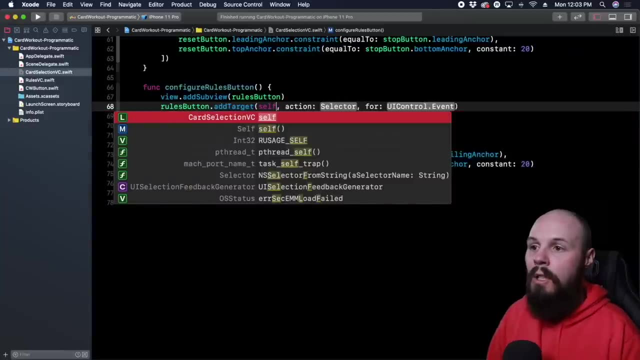 happens when the button is tapped is: we can do rules button dot, add target and you can see. we get the parameters here, the target itself for the view controller action. remember hashtag selector. this is where we have to pass in an at objc method. so let's do hashtag selector. 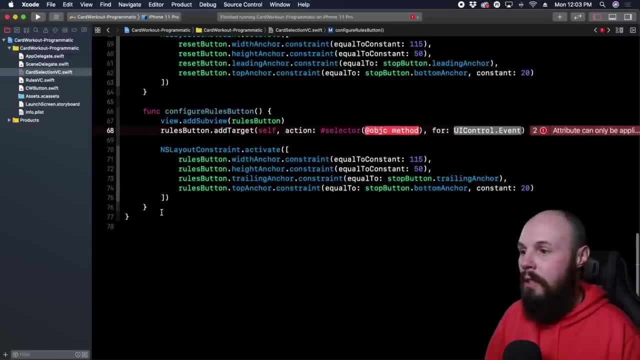 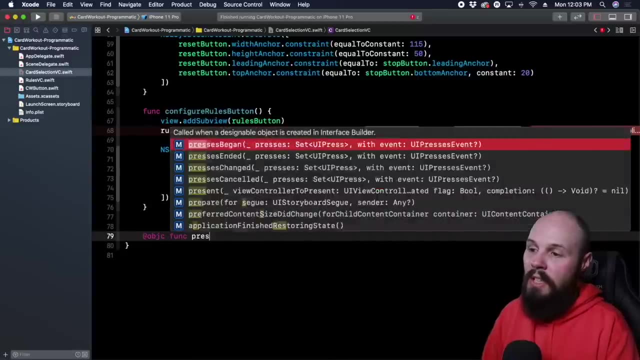 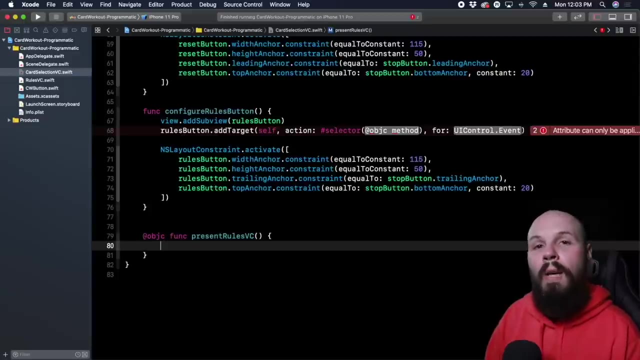 and now let's create that at objc method. here we'll do that at the bottom because this is a simple uh, present. so we can do at objc funk and we'll say: present, rules, vc. and here in this function we'll do every view controller has this function called present, which is how they present a view controller. 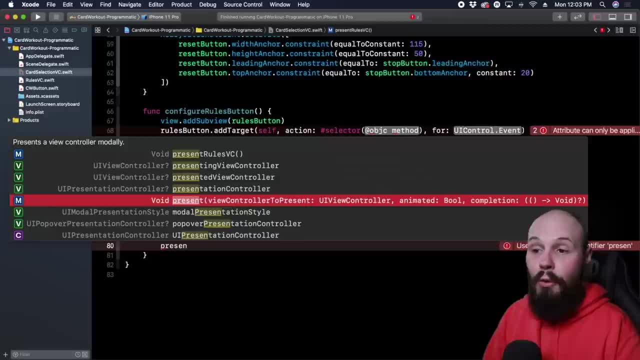 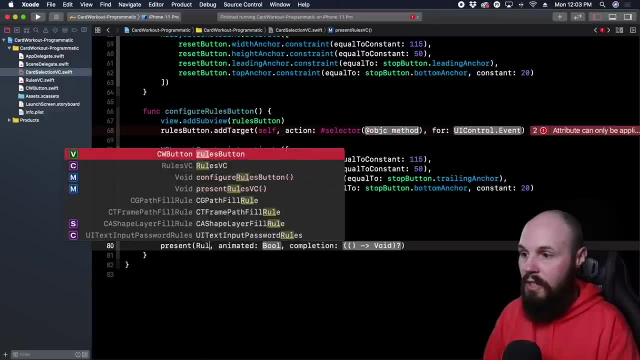 so you can see present down here and it takes in a view controller to present and you can see animated and completion hit return. so the view controller we want to pass in is a rules vc here and we can initialize an empty one more on that in a second. uh, animated is true, that means we do. 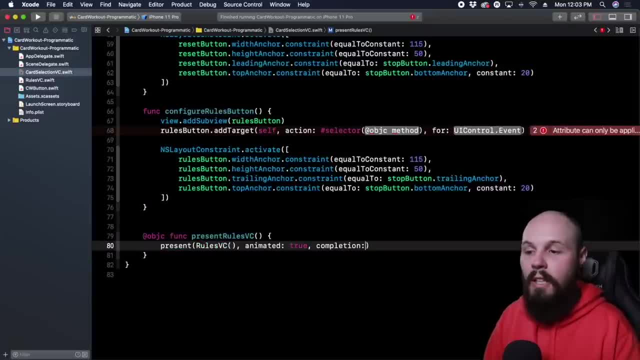 want it to slide in and we want to pass in a rules vc here, and we want to pass in a rules vc uh, and then completion handler. we're not doing anything with that, so we can actually delete that parameter. now, if we were passing data or configuring this rules vc like right now, we just 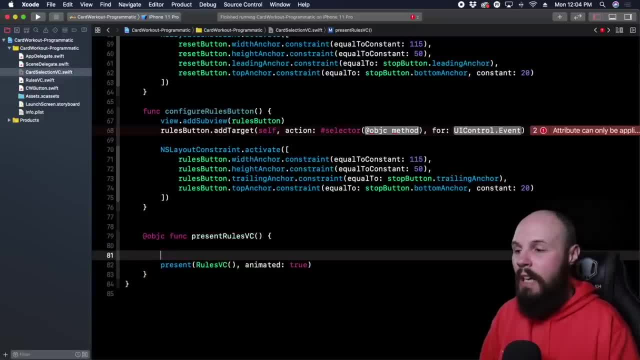 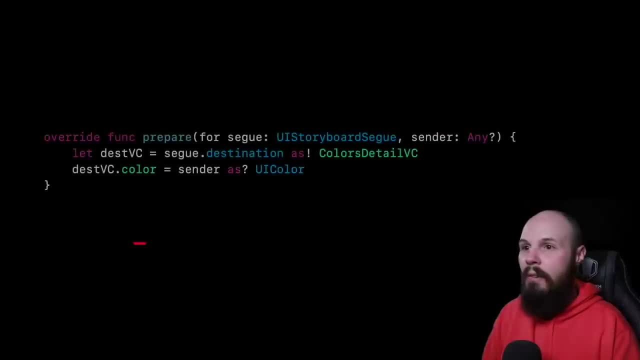 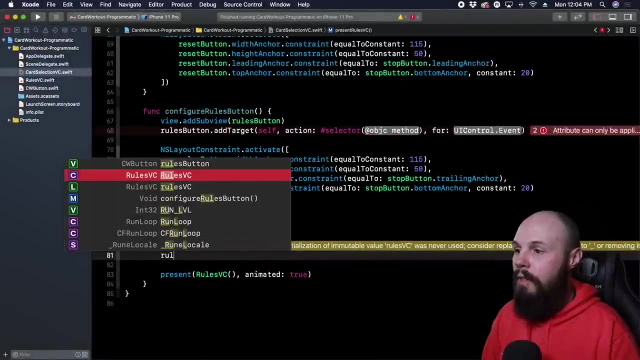 configured this, but this is kind of similar to that. prepare for segue. if we wanted to, uh, we could do. let rules vc equals. you know, initialize an empty rules vc and then remember how, on the table view, we had the variable of color uh, that we had to change. you know you would do rules uh vc dot. 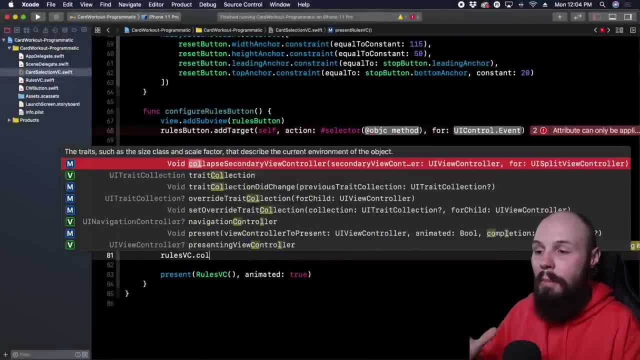 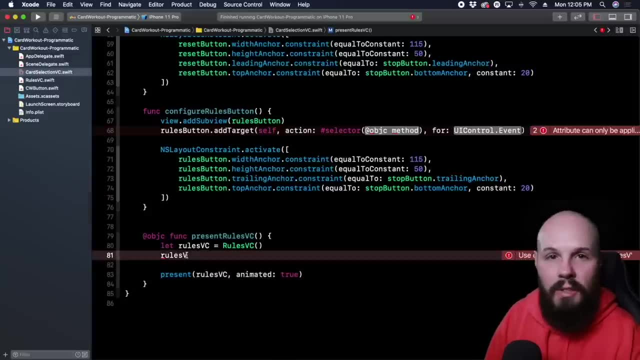 color. obviously we don't have that variable, but i'm showcasing the table view and i'm going to show you how you can pass data uh here. and instead of initializing this rules vc here, you would pass in the rules vc that we created that has like our custom data and everything like that. but again, 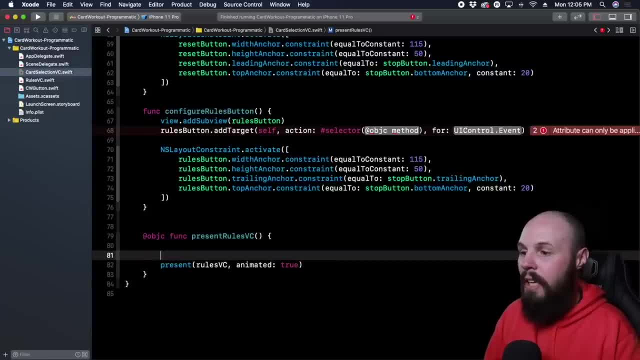 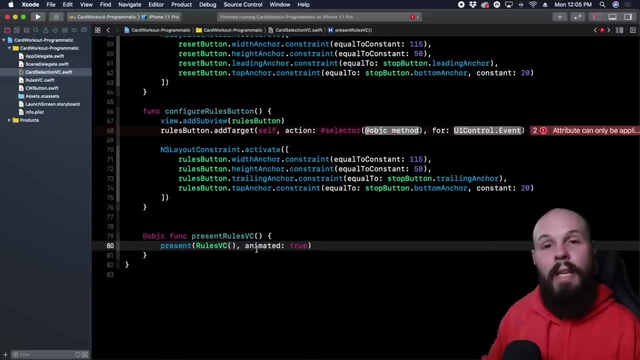 because we're not passing any data, we're not doing anything. we can initialize the rules vc right here. make it a capital r, so it's the class, and there we go. so again what this says. i know. i hope that didn't confuse you. if it did, comments slack happy to help, but we're presenting a brand new rules vc. 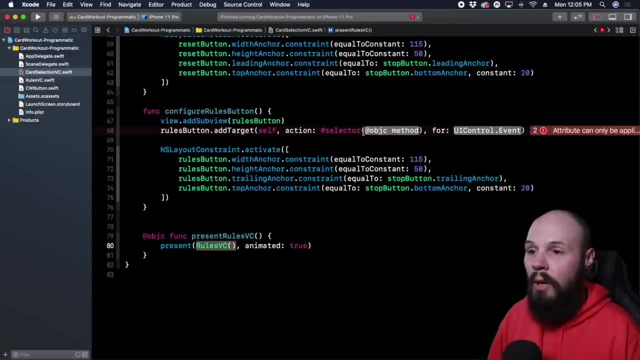 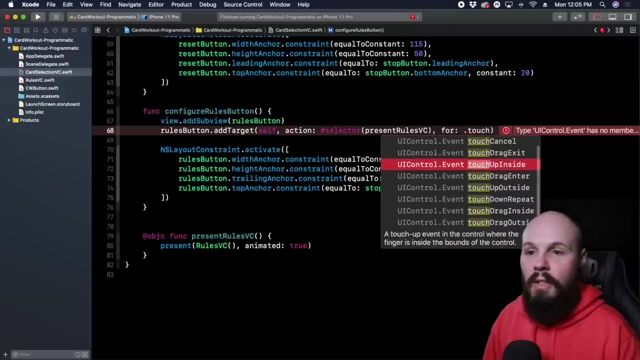 and it's going to be animated. so let's call this up here in our target. uh. let's call present rules, vc and four dot touch up inside. remember when we created our action we had to pick one of these and it was always touch up inside, like that's the uh default. so there you go, touch up. 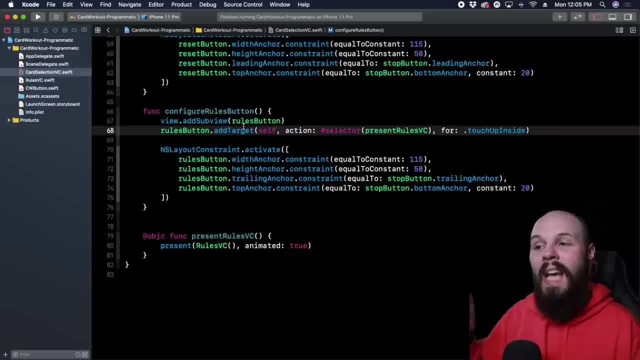 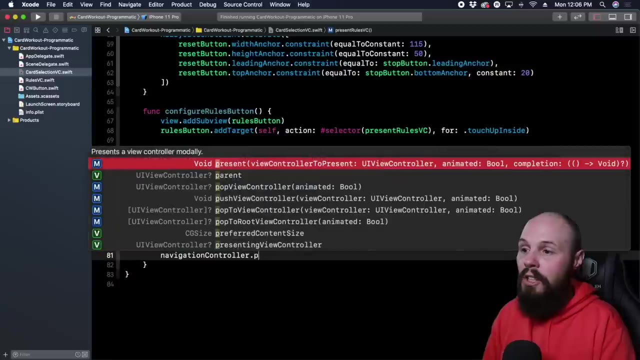 inside. so now our rules button has a target that when we tap our rules button it's going to fire off present rules, vc, and present rules vc again presents the view controller. remember, presenting is modally. if we were in the navigation controller we wouldn't use present, we would use navigation controller, dot push view controller and we would. 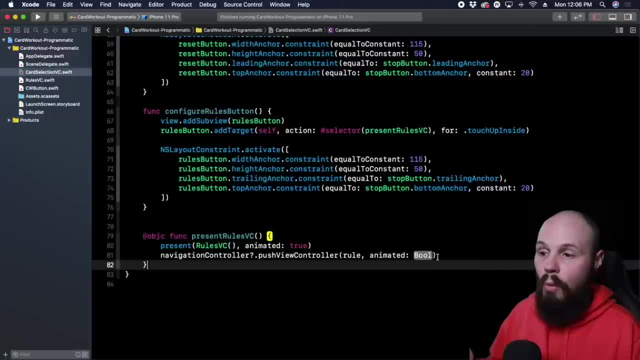 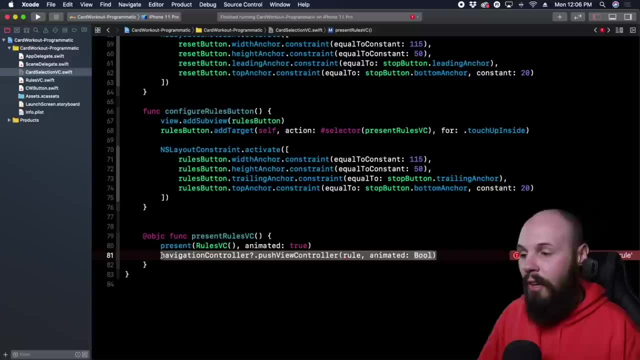 pass that view controller in there rules vc. we're not in a view controller, so this won't work. that is actually why view navigation controller is optional. right, because we're not in a navigation controller, but every view controller does have that function. but again we're presenting this. 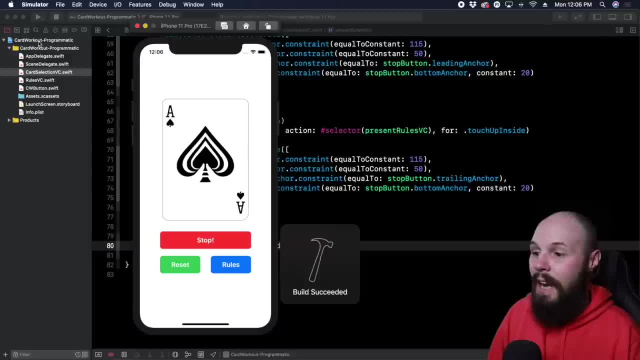 one. so it's sliding up from the bottom. so let's run it. and here now, when we tap rules, there we go, our sheet slides up and if an ios 13, we can slide it down, rules slide it down. i don't know if the simulator is not animating it, but that's a simulator issue, so let's run it again. rules there. 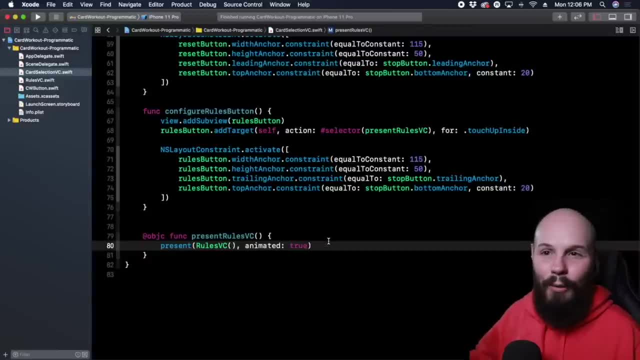 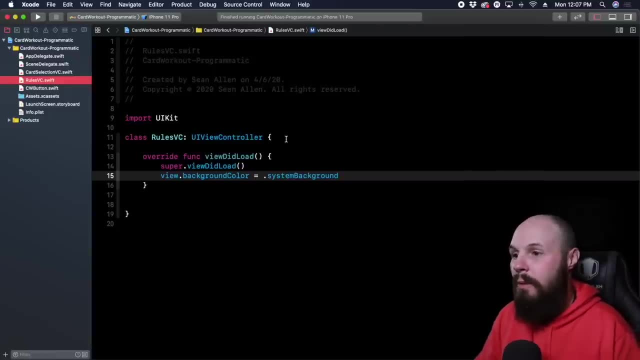 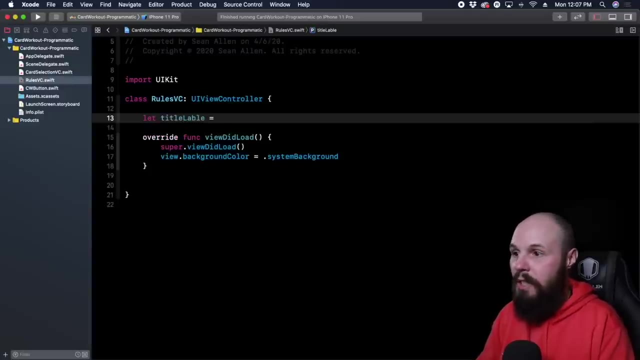 we go slide up and down. so now that we can actually see our rule sheet, let's go into our rules vc and start configuring it so when we test it we can actually see it. now, just like we did before, let's create three labels, so let our title label equal and again it's just an empty ui. 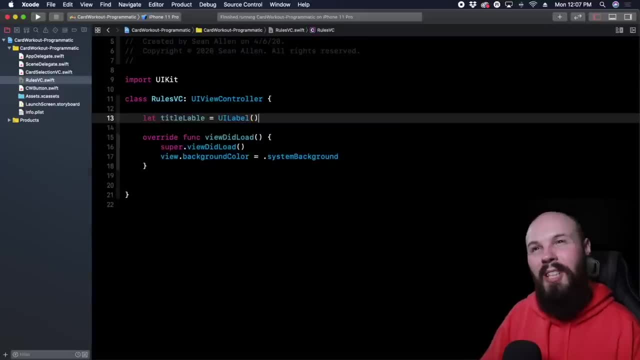 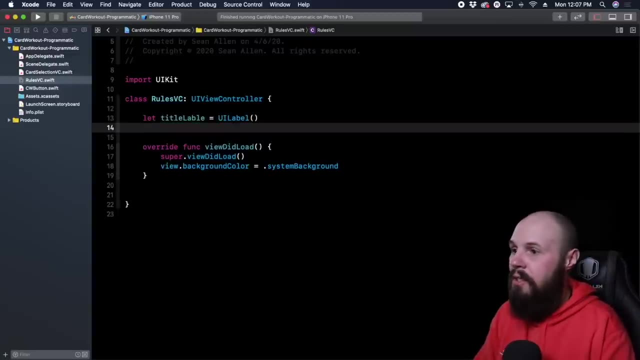 label because we didn't create any custom labels for this. we potentially could have. like, i thought about doing that, but i'll talk more about that once we have it, so let's go ahead and do that. so we're just going to use regular ui labels for this. so let rules label. i'm gonna spell label up. 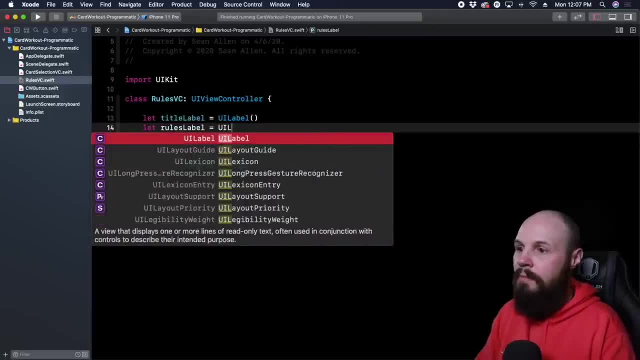 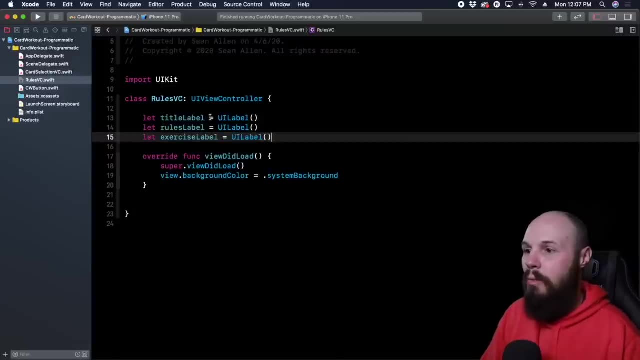 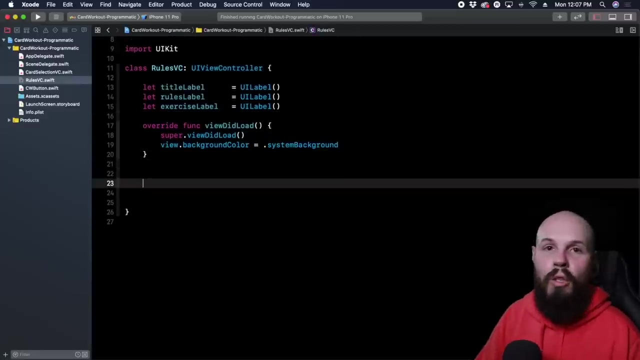 here yo uh equal ui label and let exercise label: equal ui label here. so we're just creating the objects and we'll have to configure them and lay them out in constraints- uh, later on in other functions. so, like i said, this is kind of preference. i'm not going to create that overall configure you. 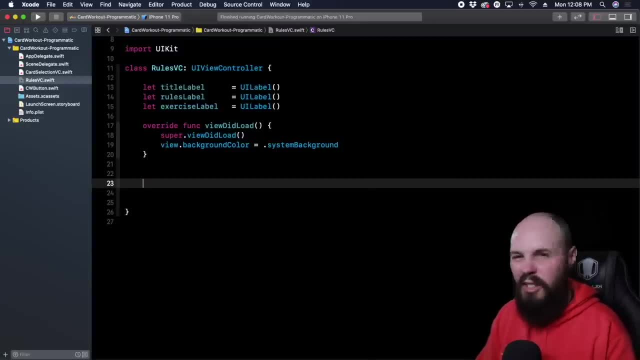 uh ui method. we're just going to configure them individually. just to show you multiple different ways to do it. use whatever you want to do it. just to show you multiple different ways to do it. use whatever you you like best. so let's do funk, configure title label. and now let's call this: 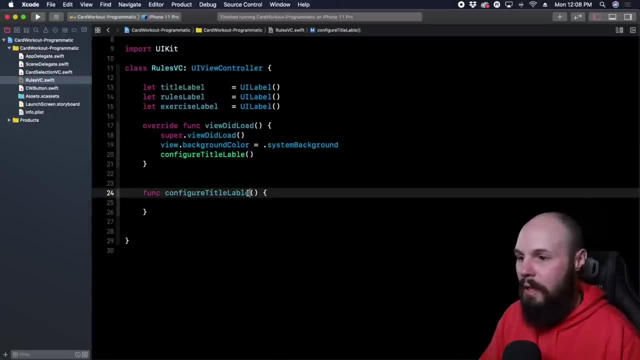 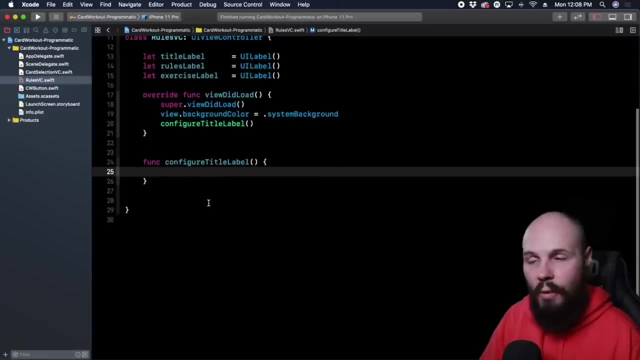 here in view to load. before i forget: configure title label. wow, i keep misspelling label bl, bl. there we go, um, and then now we do our configuration for the title label. now this is a little bit more in depth, um, but again, the first thing you always have to do, don't forget. 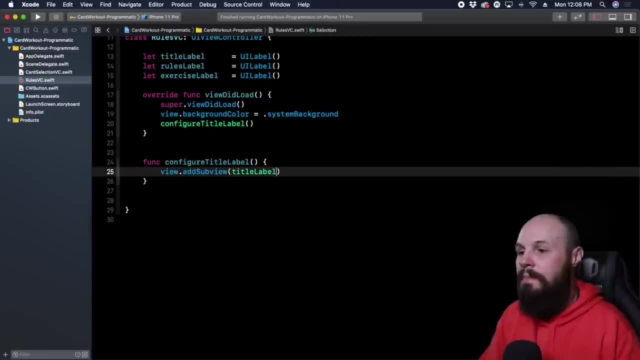 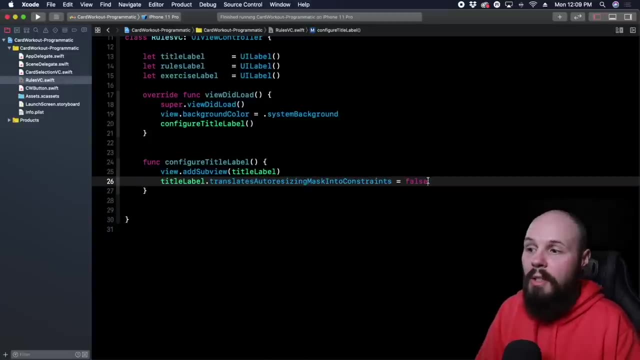 this view dot. add sub view title label and then also title label dot. translate auto resizing mask into constraints equals false. now we start configuring the properties of our title label. let's start with what it says first. so title label dot text is what it says. and if. 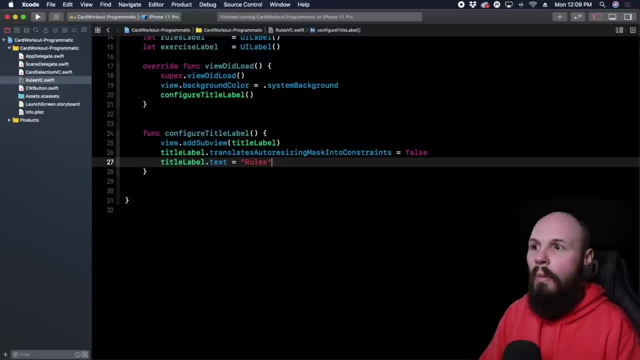 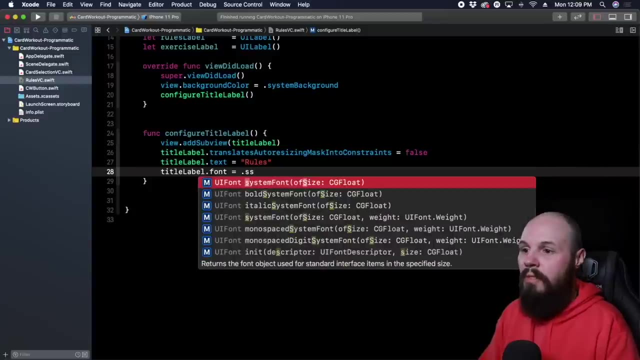 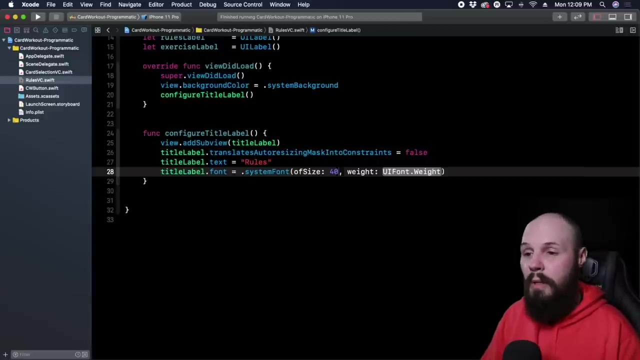 you remember this just says rules pretty simple. there we also need like what font and what font size. it is so title label: dot font equals dot system font of size. we also want weight. we want remember this was bold, so the size was 40, right, this was the big rules label at the top and the 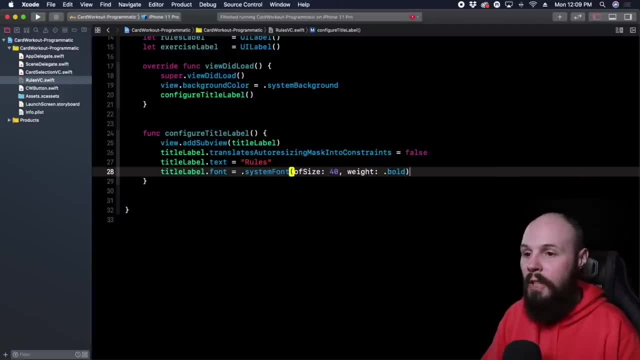 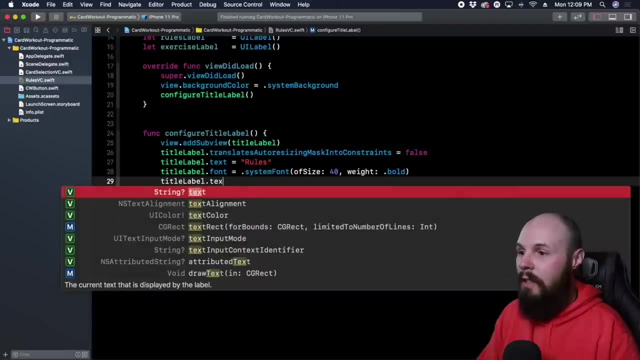 if you tap the period, you can see all the different kinds. uh, we want to be bold here. um, if you remember, this was also centered right, it's not a line left, so you can do text alignment. uh, title, label, dot. text alignment equals dot center. there we go. now you're starting to see. 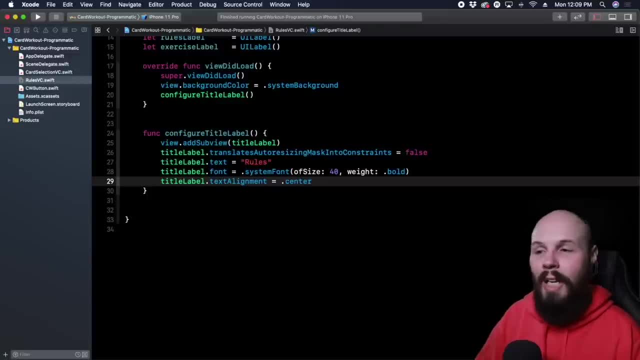 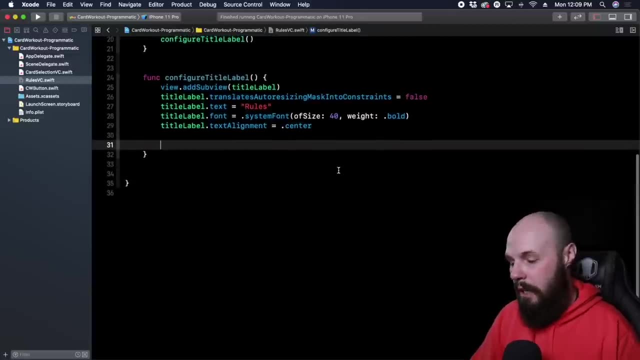 right, when you were doing this uh in storyboard, you just had all these drop downs that you could set this here. you got to set each one uh in code. so that's all the configuration we need. now let's do the constraints. uh, here we can do ns layout constraint, dot activate. again. told you repetitive. 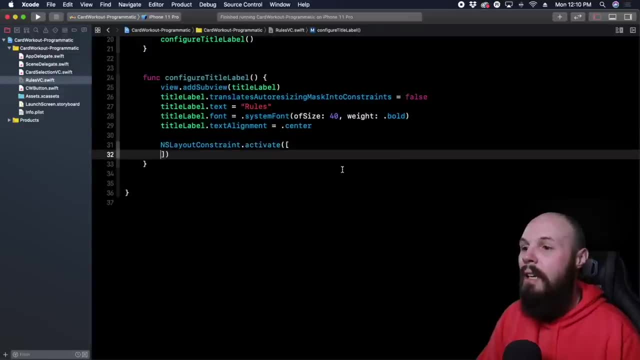 we're going to do this a lot, not curly braces, uh, just brackets. so this was, uh, i believe 50 or 70 from the bottom. i mean we can, we can tweak it and dial it in: uh title, label, dot, top, top, anchor, dot, constraint, and we're going to 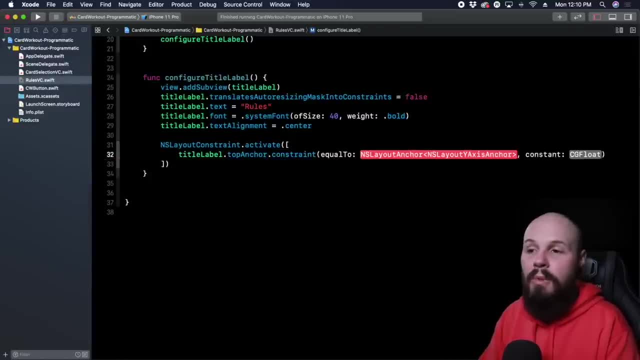 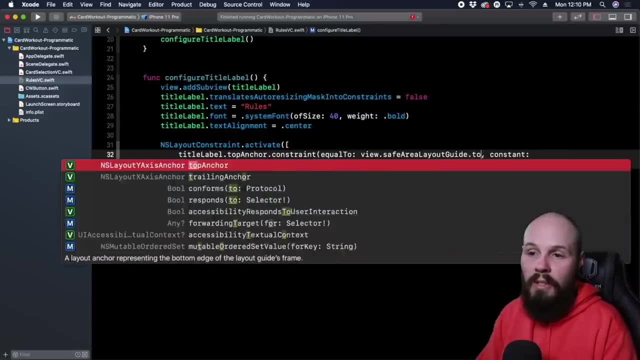 pin this to, it's going to be a little different. remember, we use the safe area, so we do view dot and then if you type safe area layout guide, you can see that. so this is pinning it to the safe area and we want to pin it to the top anchor of the safe area. and again, that's to deal with the 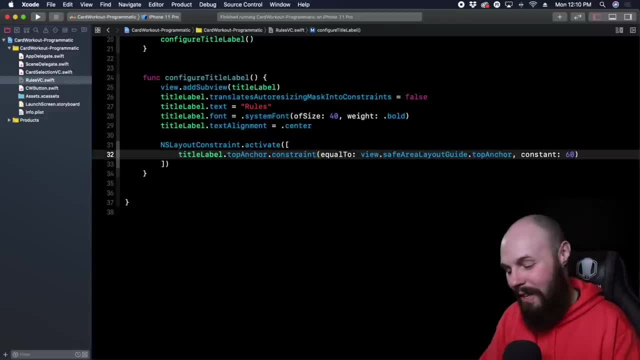 same thing, uh. so we'll go ahead and do that, put a comma in there, and you know i'll actually do that until we get to the second bracket. so we'll go ahead and do that and let's do it 50 or 60.. i cake. 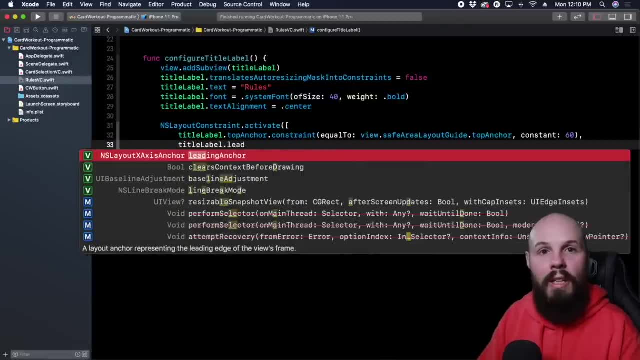 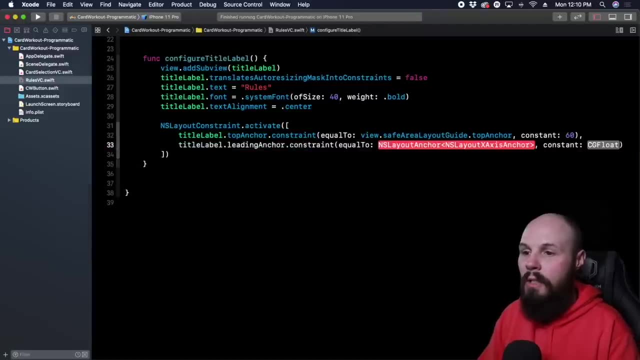 remember if it was 50 or 70, so we'll split the difference and make sure you put a comma in there, because again, this is an array. uh, so now this was title, label dot. leading anchor. remember we pinned it, 30 to the left and 30 to the right, the leading and trailing. so leading anchor dot, uh, constraint. 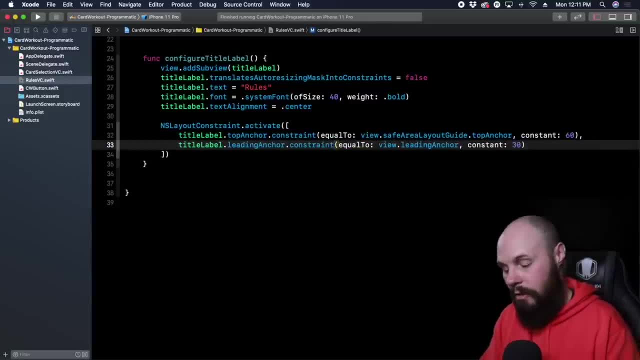 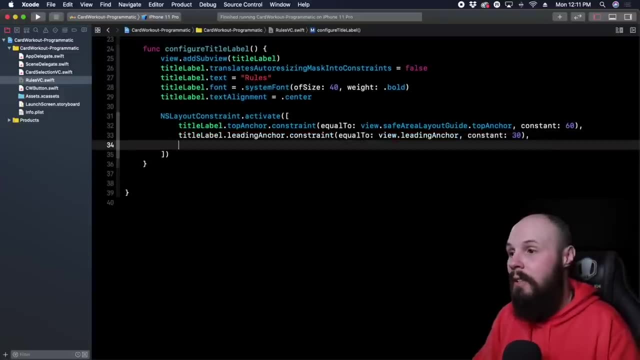 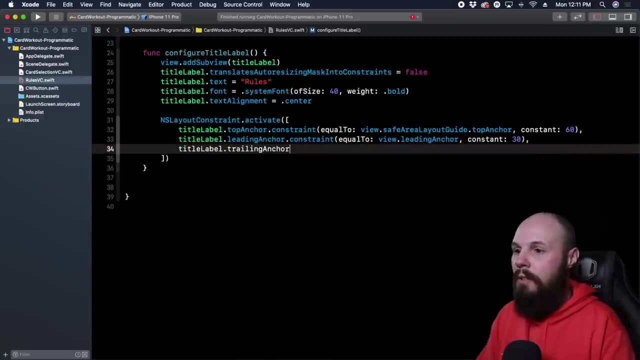 as equal to the anchor, with the constant uh view dot. leading anchor. so remember, we pinned it to the and again. this is the same thing we did in storyboard by pinning it to the left and the right. So can you think of what's next? The trailing anchor right. So title label dot. trailing anchor. 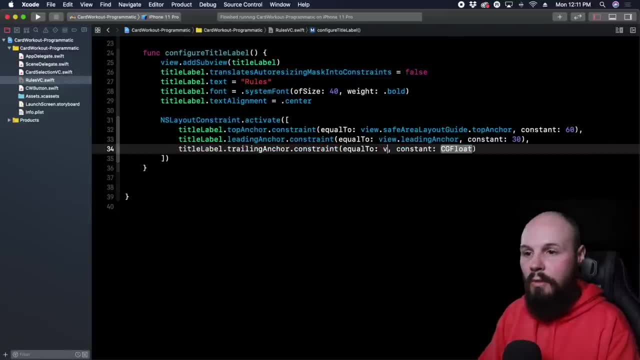 dot constraint, again equal to the anchor and their constant. so view dot trailing anchor this time. Now here's the tricky thing with trailing anchors and if you're pinning it to the bottom you have to use negative numbers. so negative 30. Remember that trailing and bottom you have to use negative. 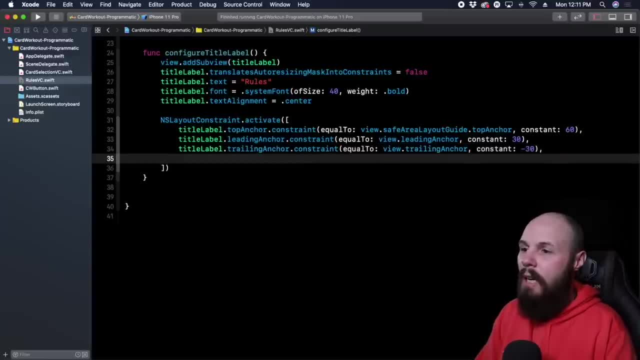 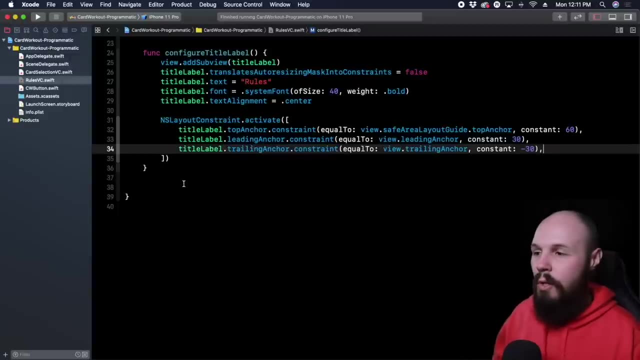 30. You have to do with the coordinate system. so now we need- no, we don't need- a height. remember, the label does the intrinsic content size, so we don't have to give it a height. so again the labels. again one of those ones where you don't need the four constraints. Remember, I said the four. 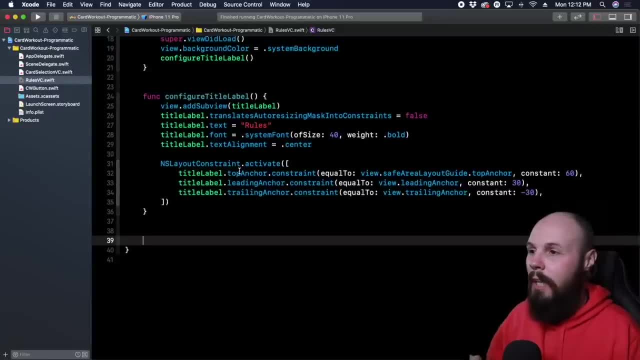 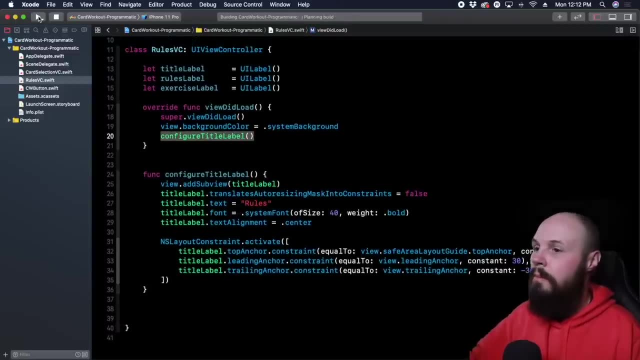 constraints was a rule of thumb that would mostly correct. this is the case where it's not So. we have our title label. we've called it in view to load. if we run this, we should see our rules title label there. So run. okay, let's tap the rules button. there we go. perfect, rules, tap the rules button. 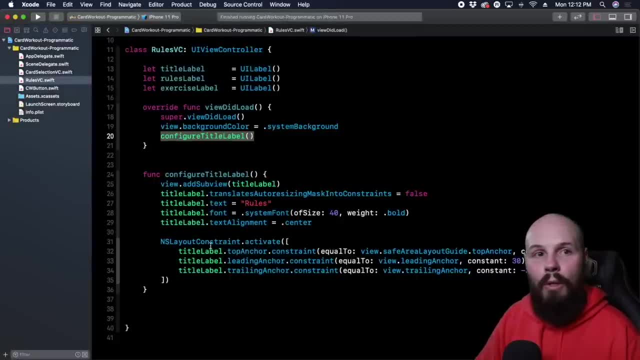 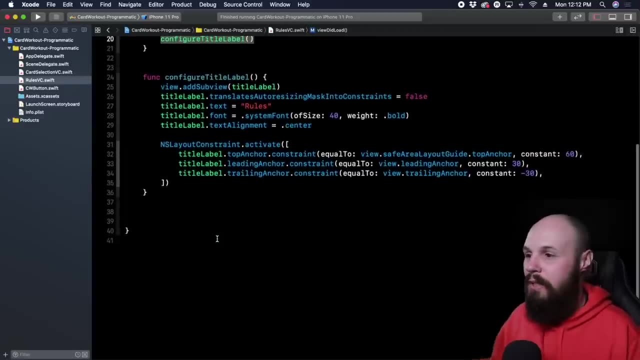 slides up rules button. slide up- cool. now we need our- I call it the rules label, because that actually tells the rules. and then we have our exercise label to do, which shows you know what a heart, diamond and spade represents. so let's start doing those. we just need to. 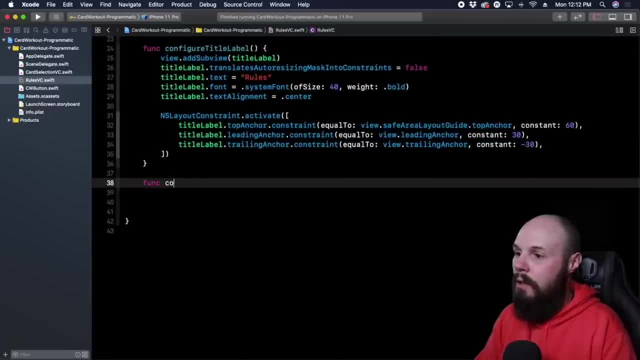 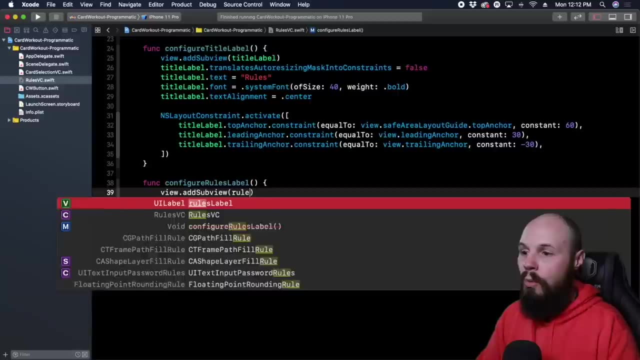 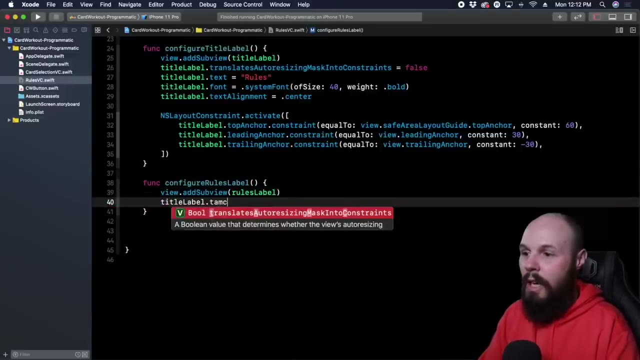 configure two more labels, so funk. configure rules label: same thing: view dot. add sub view: rules label. got to make sure we we're dragging it onto the screen and dropping it again. set the Tamek dot, Tamek. you can start actually type Tamek and it'll it'll do. it equals false, remember if you forget that line. 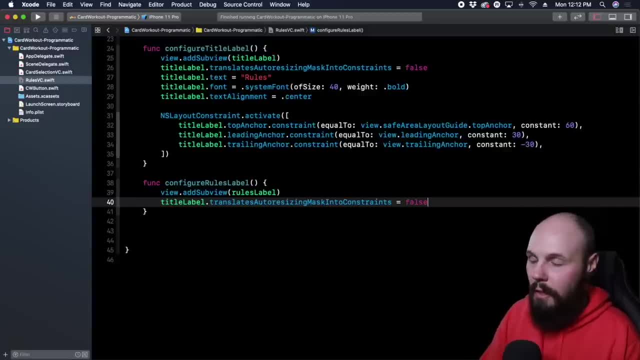 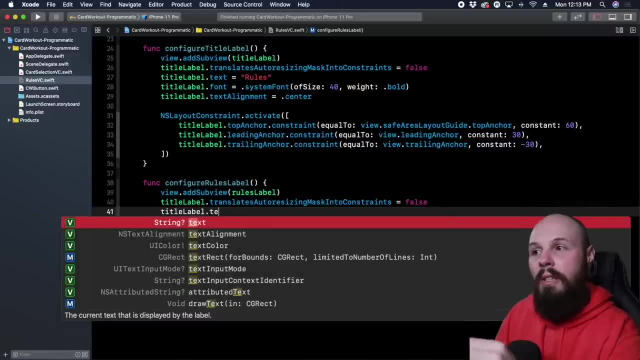 of code. your, your layouts gonna be all messed up and, trust me, you will forget that line of code. let's talk about the text now. so title label, dot text, and I'm using the, the title label. that's kind of like my structure here. I'm just going. 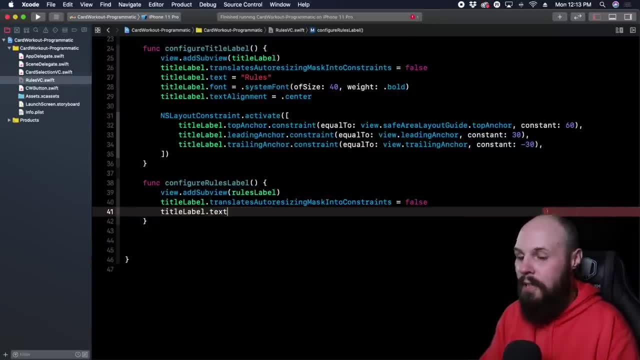 kind of going down the line to make sure I'm hitting what we need. so dot text. now this text is a little longer. the value of each card card represents the number of Xer size you do. and now here's how you do a line break. if remember in storyboard we had to hold ctrl and hit return to get the. 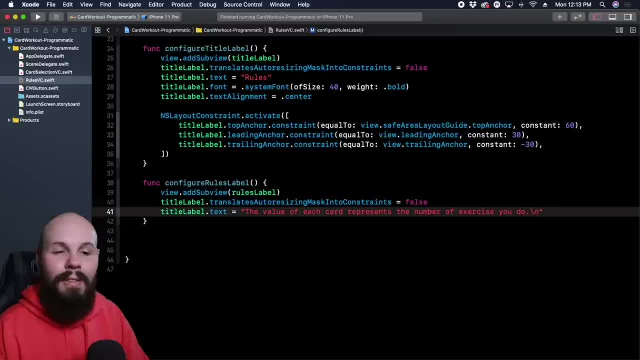 line break in our text so you can do forward slash and, to be honest, it's not forward slash or backslash. I get those mixed up right because depends on how you look at it right it's going down and forward to the angle or it's leaning. 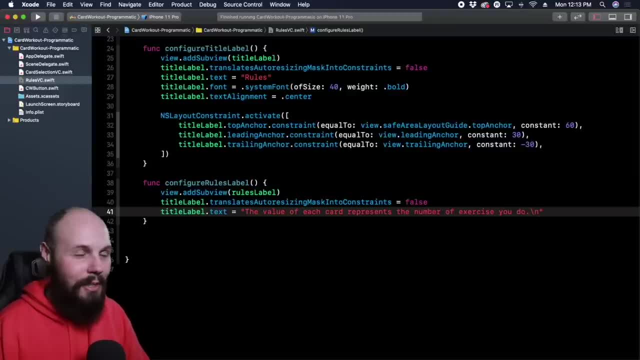 backwards, I get a mixed up. if it's a backslash and I called it forward slash, my bad, that's a. it's a 30-year habit I've got. so forward slash in, forward slash, that will give us one line break. we want to add two line. 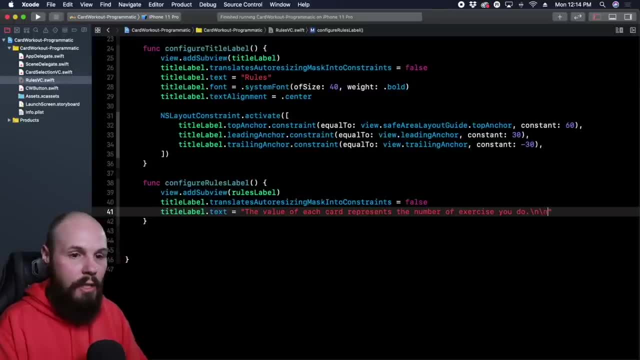 breaks in there to give us a space. so now we can do the and it's going to line wrap here. this is: jack equals 11 comma space. Queen equals 12 comma space. King equals 13 comma space. ace equals 14. scroll up a little bit there so you can see. 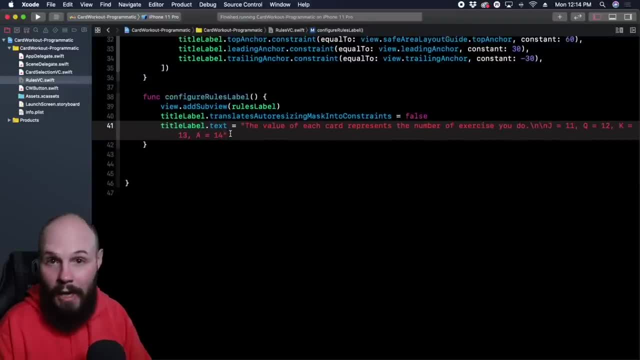 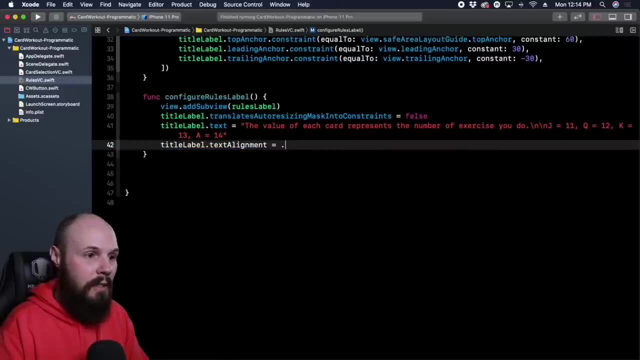 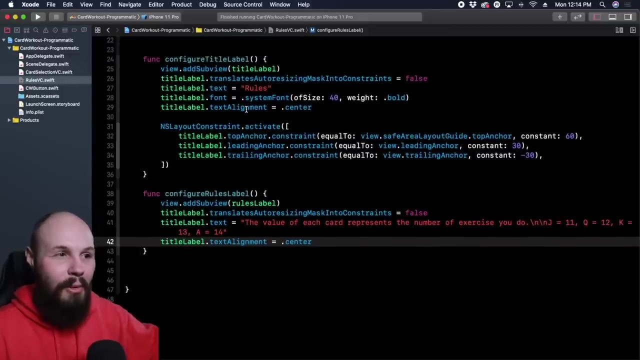 so that is our text. now we want to text align right, we align the center. so title label: dot. text alignment equals center, dot, center, not just center, uh. so that's all we had here for uh, the oh. no, we forgot font. remember, that's what i said. i always look at my other labels to make sure i hit. 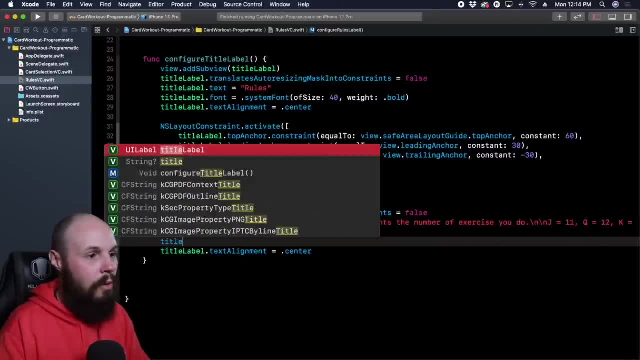 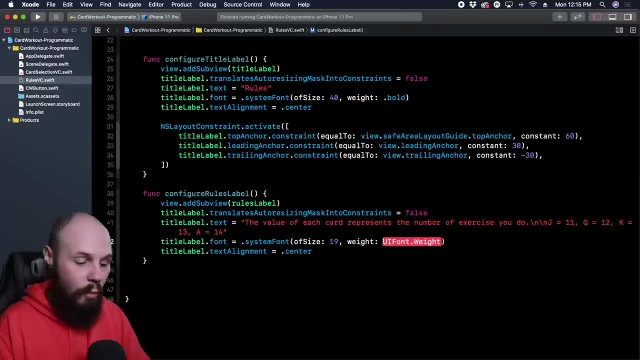 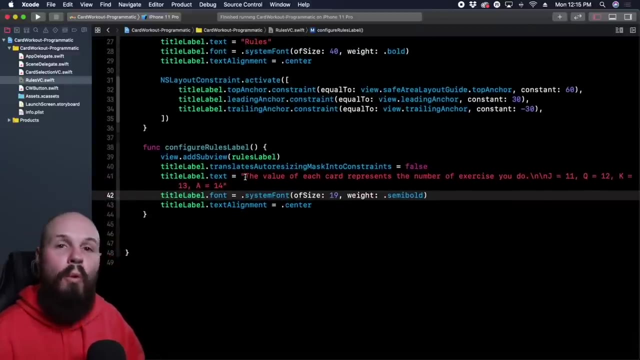 everything. so let's put font here. so title, label, dot font, and again that's going to equal dot. system font of size and weight. this was size 19, if you remember, and the weight was dot semi bold. it wasn't bold. okay so, but because this is two lines, remember, we're missing that number of lines. 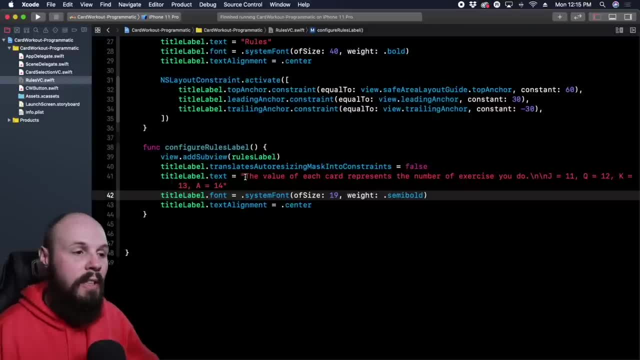 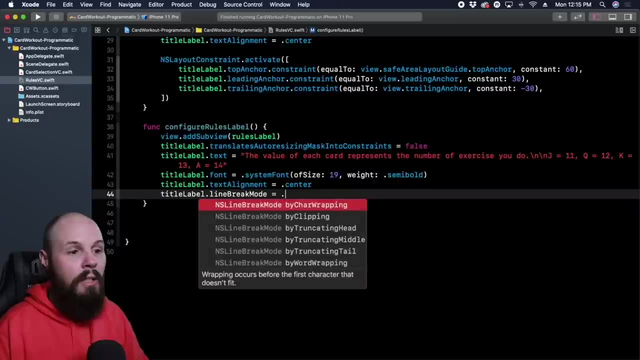 right if you just leave a default number of lines is one, and then it'll truncate the tail. so here we can do two things right: title label dot. line break mode equals dot. remember this was by truncating tail or by word wrapping. we have to set this to word wrapping, so it'll wrap based on. 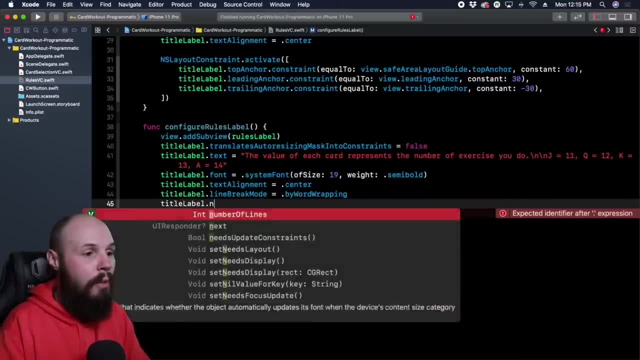 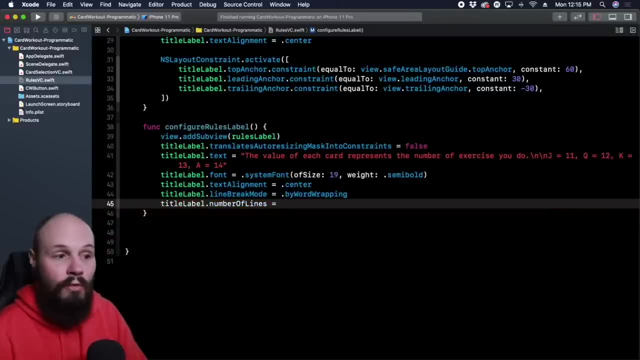 the word and then also number of lines, title, label, dot. number of lines equals zero. remember when we did zero. it'll automatically adjust if you wanted to hard code it. so it only shows four lines and then truncates the tail like if somebody wrote a huge, long paragraph. that's why you would do four. but 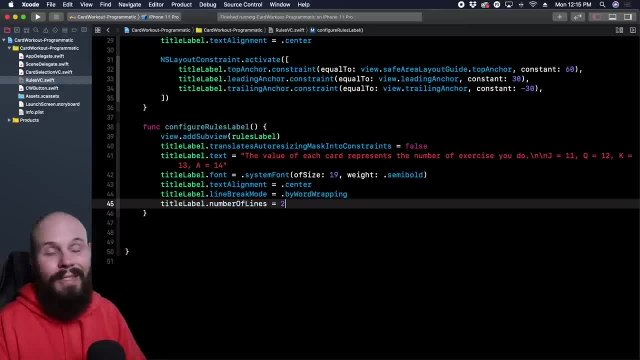 we want zero. we want this to adapt. technically we could hard code it to two because we know it's two lines, but you know we'll do zero. so it automatically adjusts. so that configures our rules label. nope, we didn't do the the constraints. so that configures like all the custom stuff we. 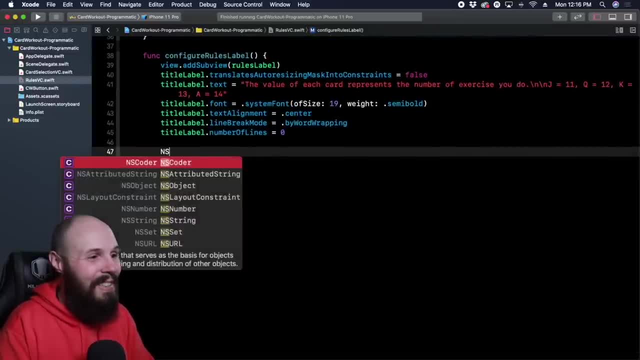 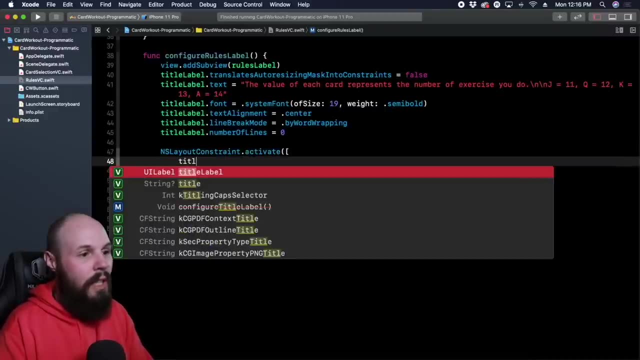 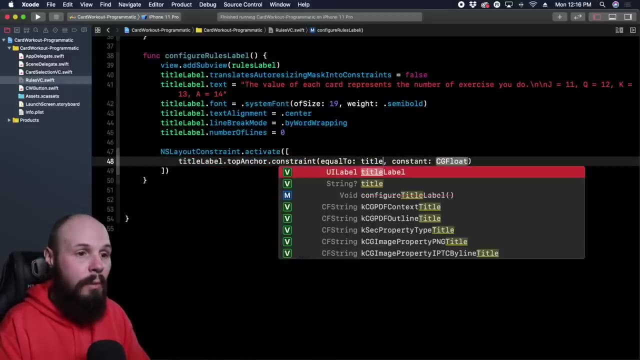 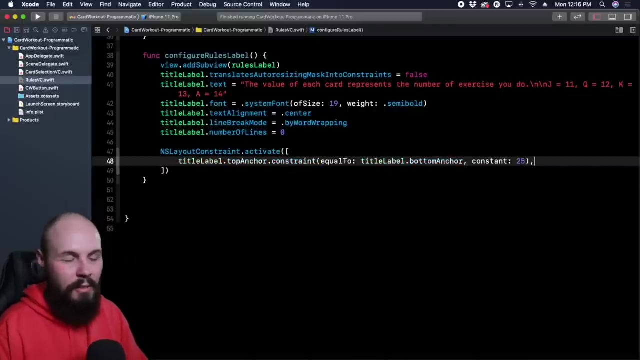 need to do. but now again, repetition: ns layout constraint dot activate and start passing in this array here again: title label dot top anchor, dot. constraint it's equal to is the bottom of the rule of the title label. so title label, dot bottom anchor and that constant, uh, i believe was like 25. i might be getting these wrong, but it's roughly. 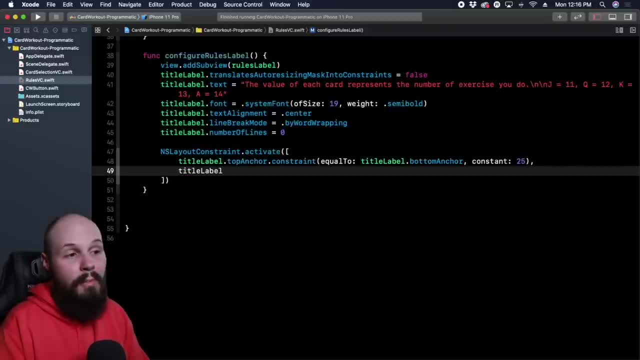 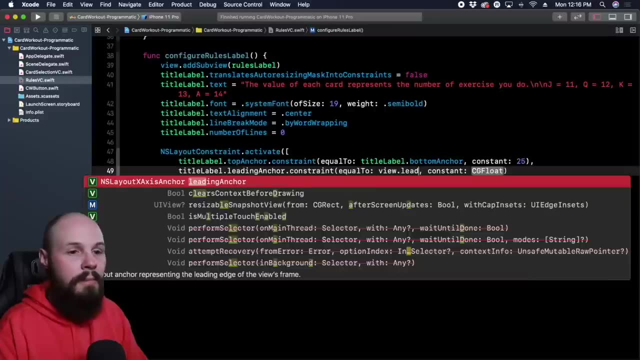 the same. it's not going to make a difference. uh, title label. remember, we did the same thing. leading anchor was 30 and trailing anchor was 30, so dot, constraint view dot. uh, leading anchor equals 30 comma. oh, i keep doing title label. wow, good, good catch, sean. i wonder. 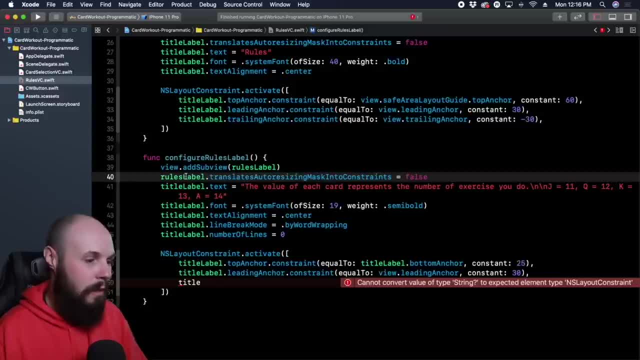 if anybody caught that this is actually rules label and command c, command v, double click, command v, double click, command v again, i could have held option, i could have done rename, all in scope. so many ways to change this again. i'm in this habit, i'm quick at it, i just do it that way. 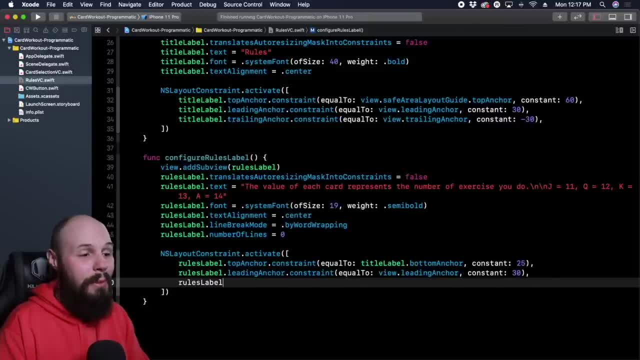 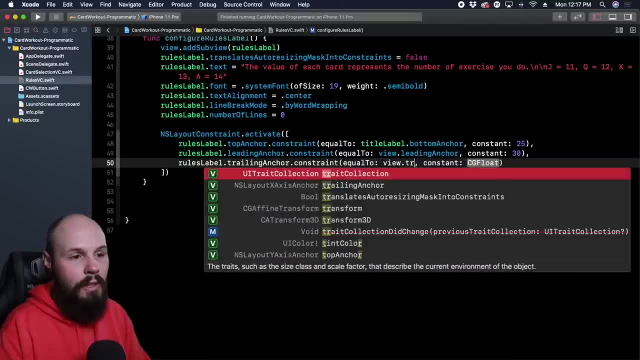 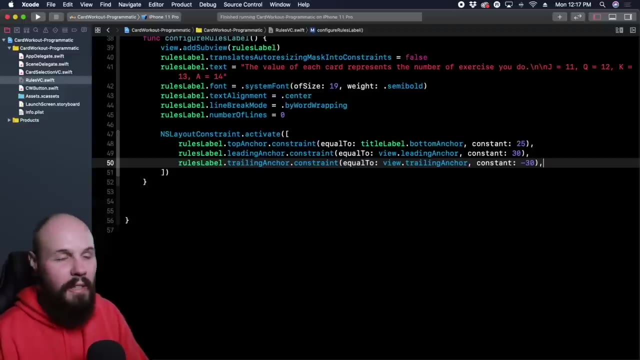 so, wow, i was doing title label the whole time. this is the rules label: dot trailing, uh anchor. let me scroll up here: uh constraint equal to view. dot trailing, uh anchor. negative 30. again. remember i said silly mistakes, programs do it all the time because you see, this is like repetitive mind-numbing code. 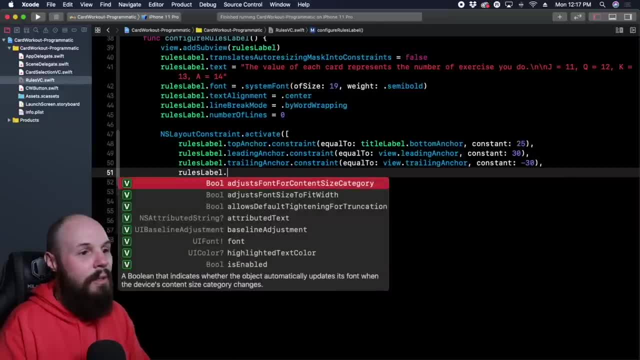 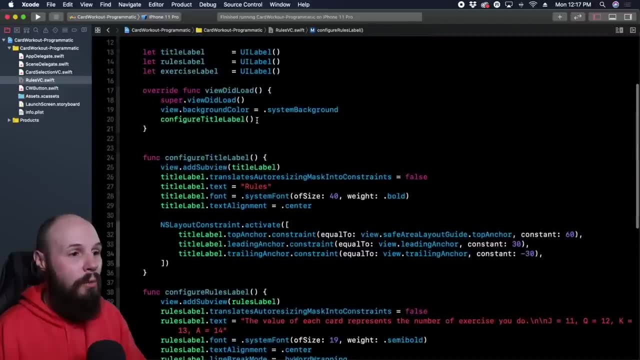 very easy to make mistakes like that. so rules, uh, labor label- nope, we don't need a height. again, intrinsic content size with the label. we don't need a height. so let me make sure i call configure rules label up here in view to load configure rules label and let's run it. and we should have. 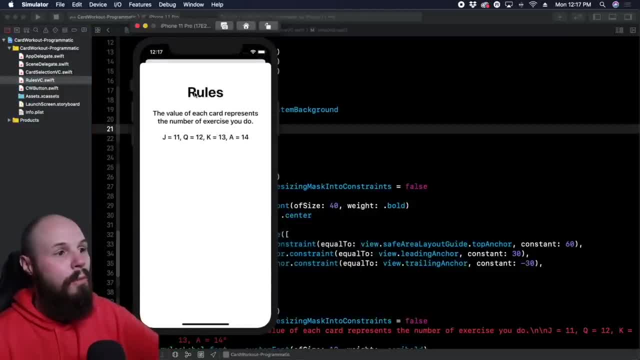 our rules label in place now, uh, below our title, yep, rules title. the value of each card represents the number of exercises you do again, jack queen king ace, cool, cool, cool. the last thing we need is our exercise label that shows what a spade is what. 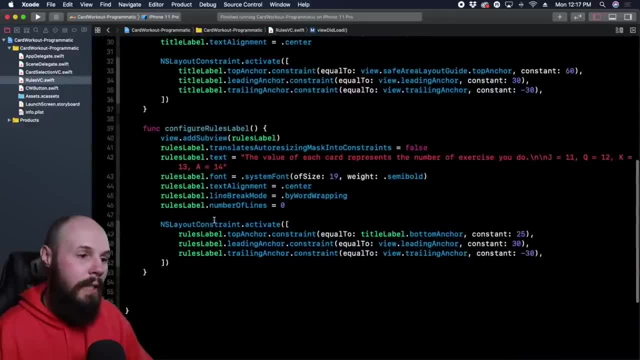 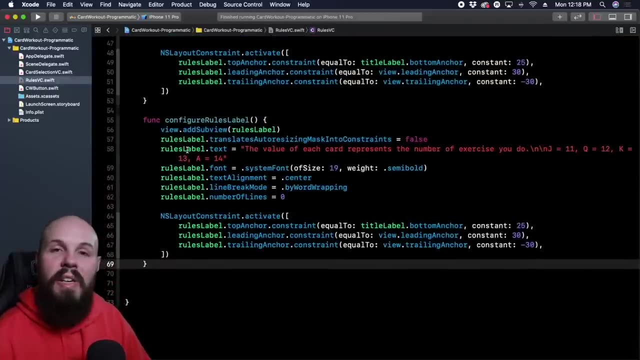 a diamond represents and all that stuff. so let's do that now. again, i'm going to use some copy and paste because you know what it's quicker. so again, be very, very careful when you do copy and paste. make sure you go line by line. so this is no longer configure rules label, this is configure exercise. 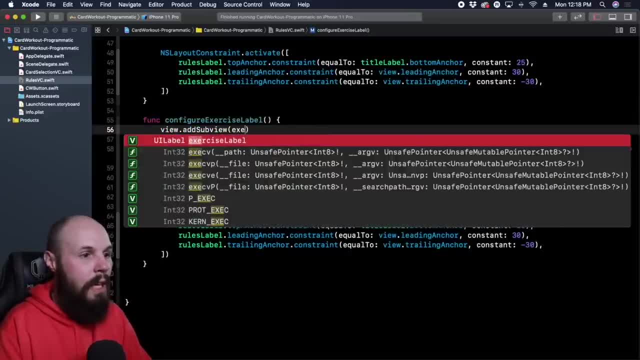 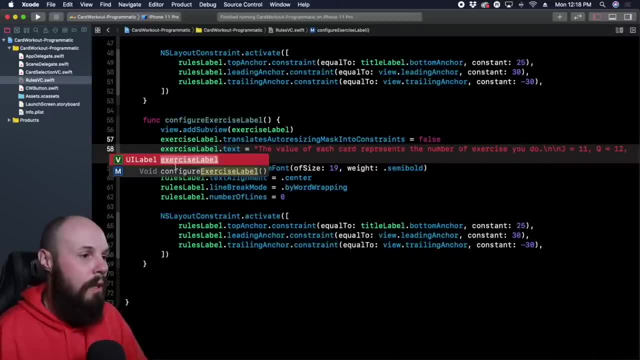 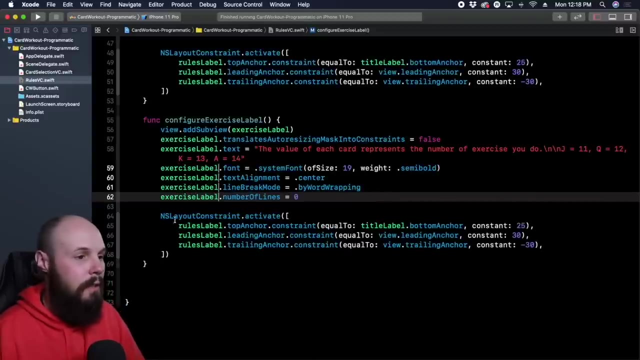 label again. view dot. add sub view, not rules label, exercise label and hold option: highlight these. exercise label, hold option again. i know people are sitting there yelling at their screen: use, edit, all in scope. i know, i know, i know bad habits die hard. exercise label: okay, so we just renamed all those. however, we're gonna have to go line by line. 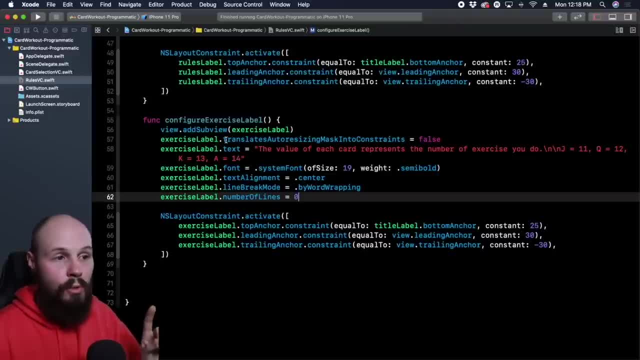 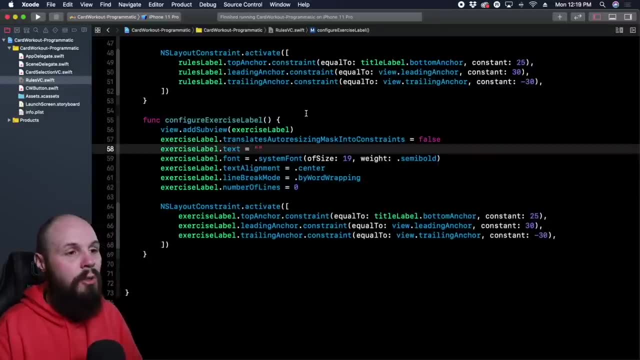 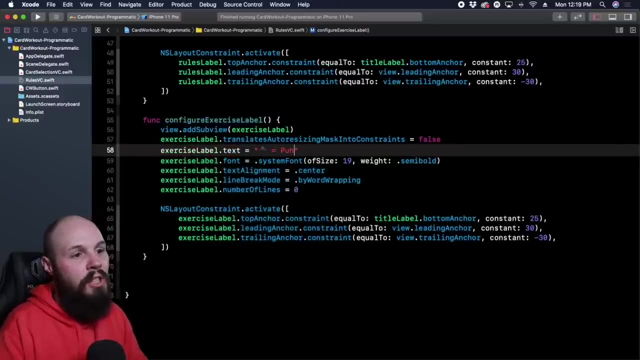 to make sure we have what we need. so exercise label: tamic. yes, we need that exercise label text. now, this is different uh, so let's delete this. so again, command control space to pull up your uh emojis- my frequently used spade. spade space equals push ups, and then four slash n, four slash n again. 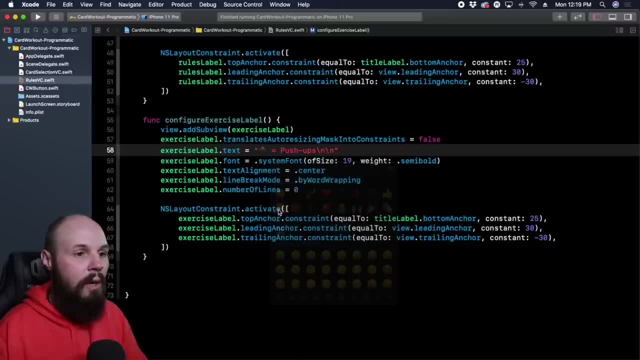 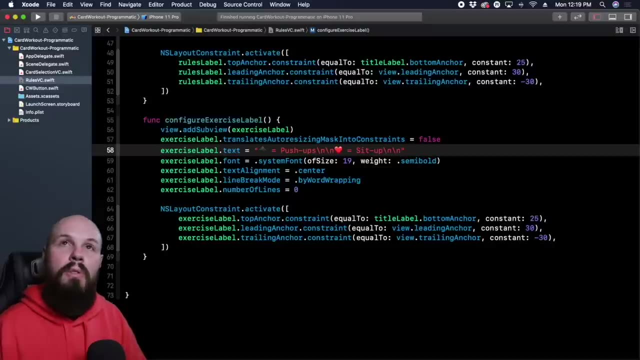 to get that extra space. uh, command shift space to get the heart space equals sit ups again. four slash n. four slash n. there are ways- i believe it was introduced in swift 5- to do multi-line strings for something this simple. i just prefer to do this um, but there are ways to do multi-line strings. maybe you want to. 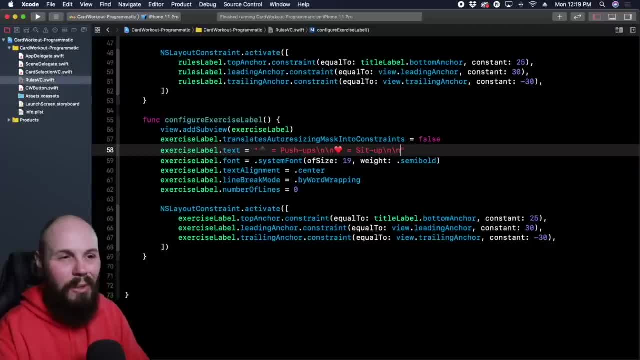 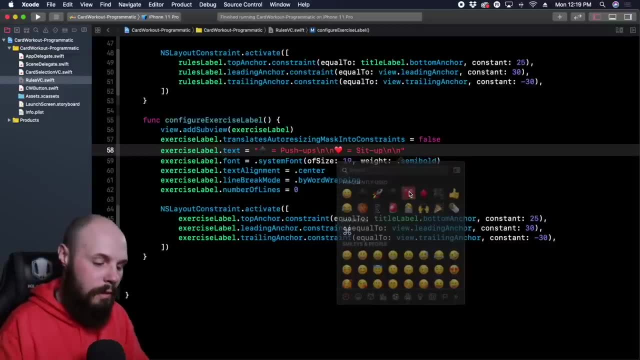 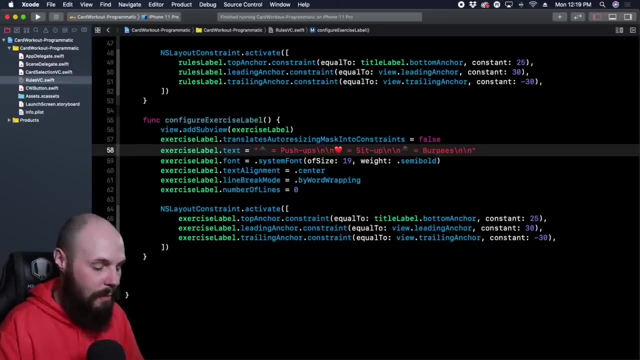 google that that was new in swift 5.. for something again, something so simple and short like this. i just prefer this: uh. so sit ups. and now we need clubs. space equals, this is uh burpees. and again forward slash n, forward slash n, and this is diamonds. 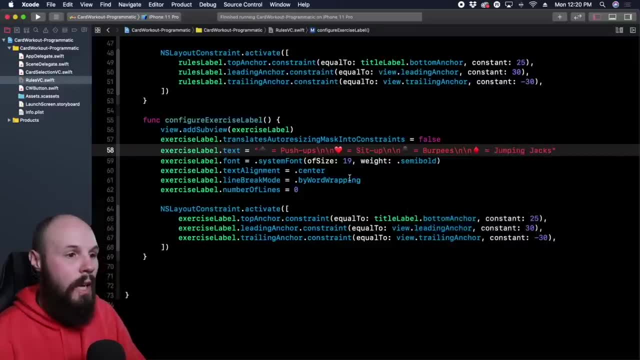 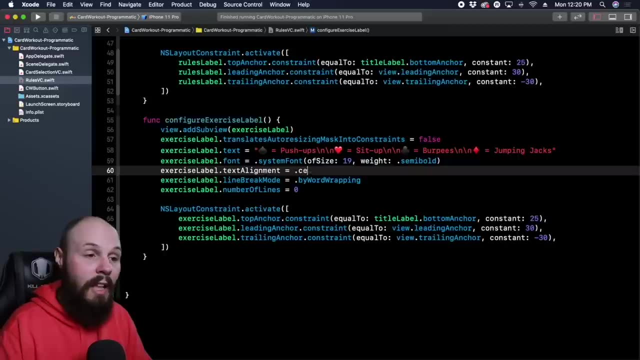 and equals jumping jacks. okay, so now, uh, the system for uh. this is the same uh font that we used to have uh normal font. i only used a normal font, auto font. this is what i started with, and then you can actually use it multiple times. uh same, this is the same. so, uh, text alignment was a little bit different to the default font. 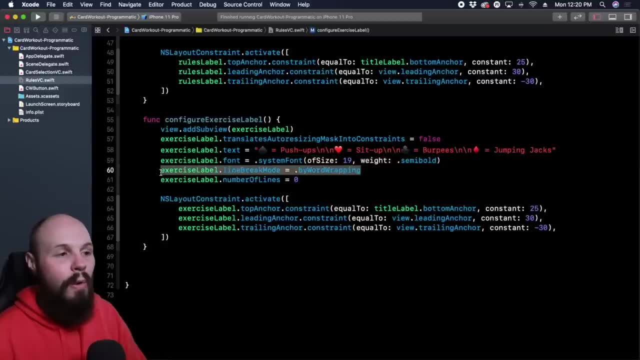 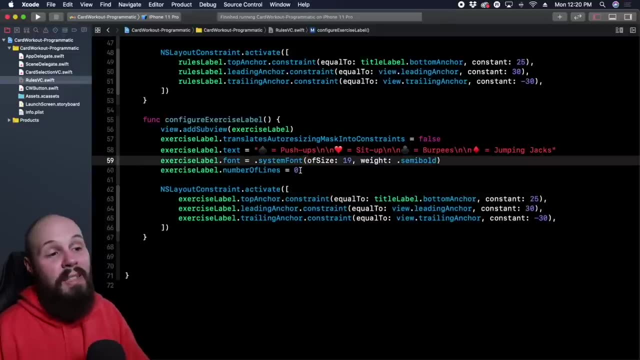 uh, font was 19 semi-bold, that was the same. uh, text alignment was not center. text line was actually left and, to be honest with you, we can actually delete this line because left is the default line break mode by word wrapping. uh, we didn't. we're not word wrapping this. where there's. 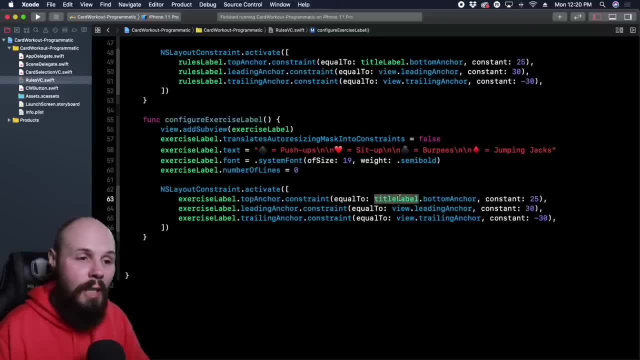 no line breaks on this label. because we're hard coding things, because we always know it's going to. We wanna pin it to the bottom of the rules label and say 25, keep it consistent. Now this label is not actually pinned. 30 to the left. 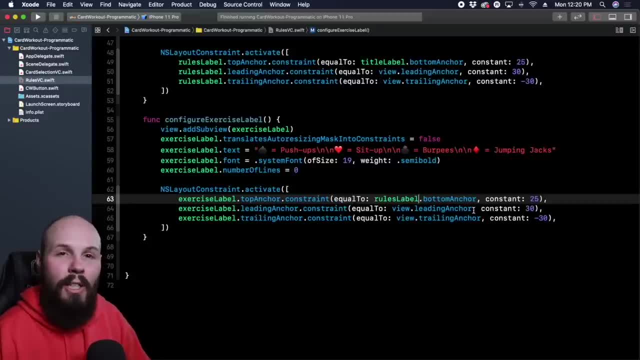 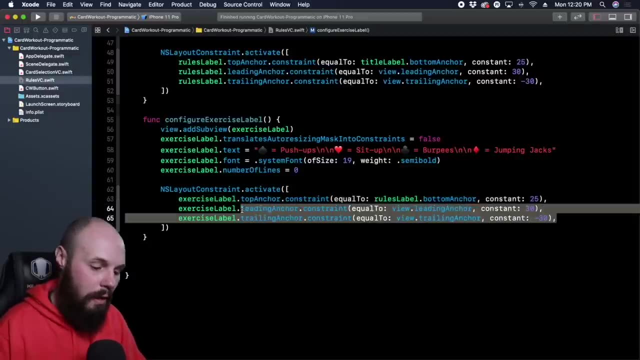 and 30 to the right. Remember we hard coded the width because we wanted to place it at a certain spot, visually to the eye, but that was just all design. So let's actually delete these constraints and do the width anchor that constraint equal to constant 200 comma. 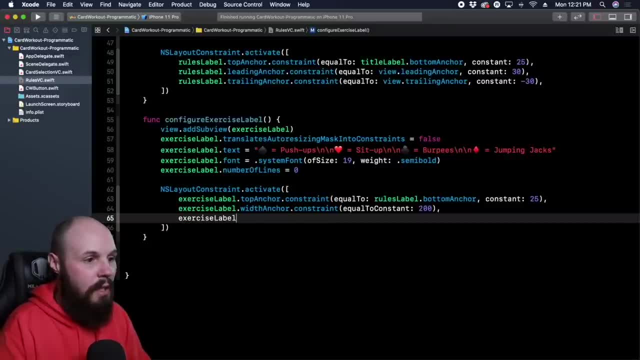 and then we centered it X on the X axis. So exercise label dot center X anchor. dot constraint is equal to view dot center X anchor And we don't have to give it a height because, again, number of lines is zero. intrinsic content size. 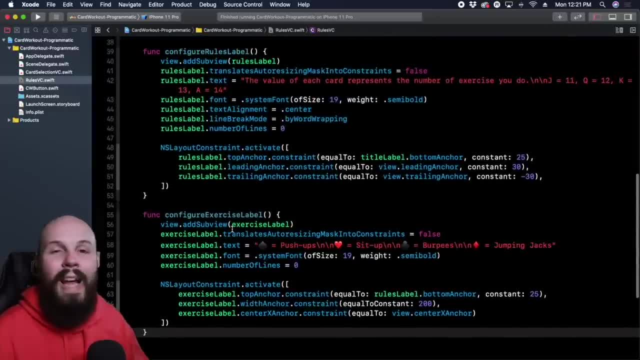 Now I do wanna say something. when you're dealing with labels- we're not gonna get into this in this exposure beginner course, but I don't know if you're familiar with dynamic type on the iPhone, where people can change the size of their text. 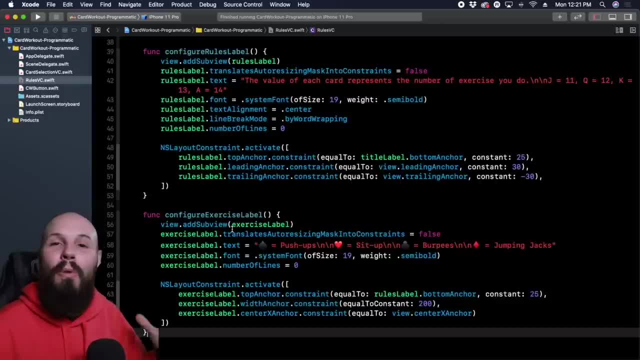 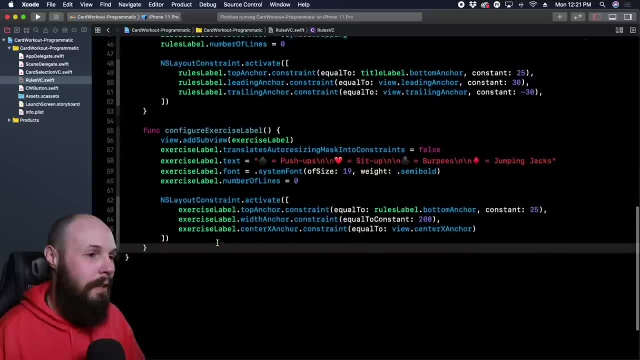 Like: have you ever looked at somebody's phone and their text is all blown up? Well, you have to be real careful to handle that with how you lay out your UI and your labels. That is way beyond the scope of this beginner course, But if you do have experience with that, 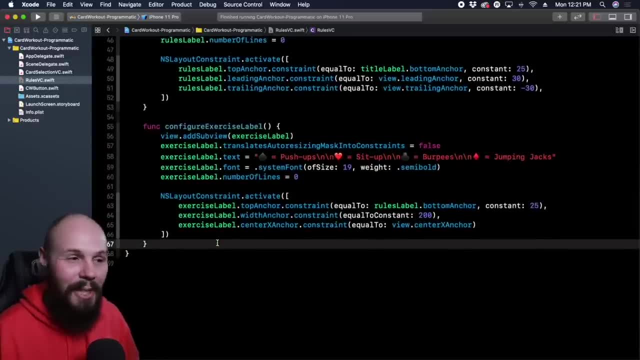 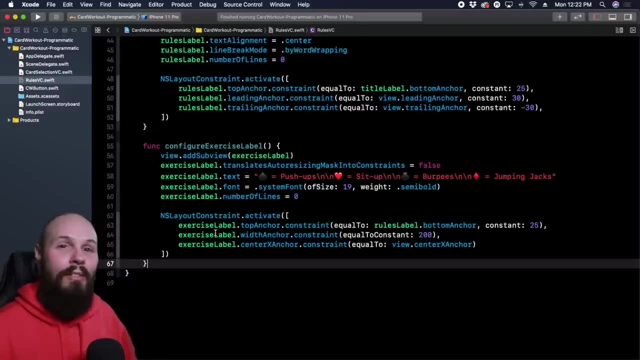 and you're like: hey, you didn't handle dynamic type, Like I know I get it, we're just not doing that. yet Again, you have to learn to crawl before you can walk and then walk before you can run. Like I said, this is a process, this is an evolution. 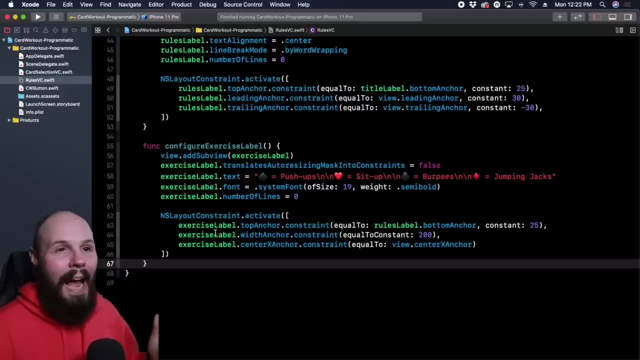 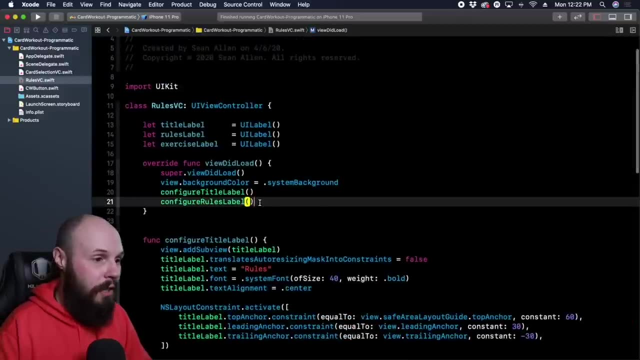 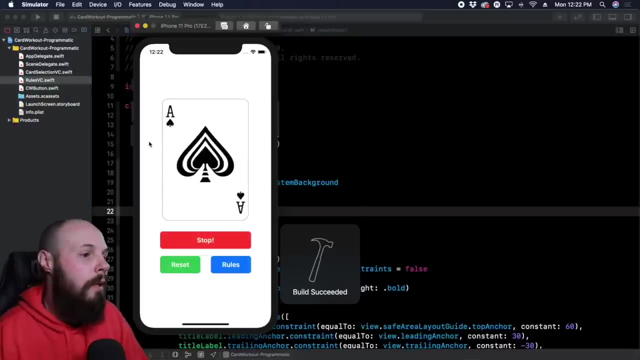 This is just your first exposure, But again, that does illustrate like how deep app development actually goes. Like it's pretty deep and we're just scratching the surface here. So let's call configure exercise label and then we're gonna go ahead and run it on our iPhone 11 Pro. 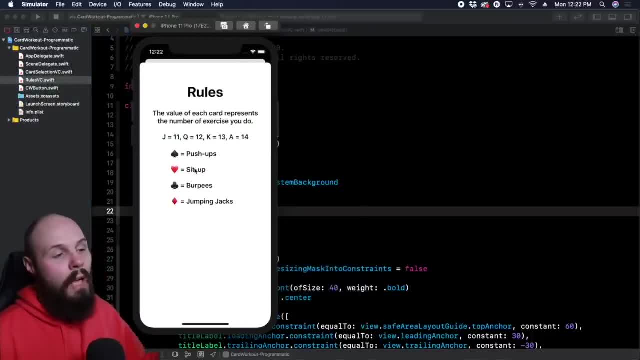 Hit rules slides up. Cool, now you can see this Now. okay, I messed up, We did 25.. We pinned the top of this exercise label 25 from the bottom of our rules label. To me that feels too cramped. 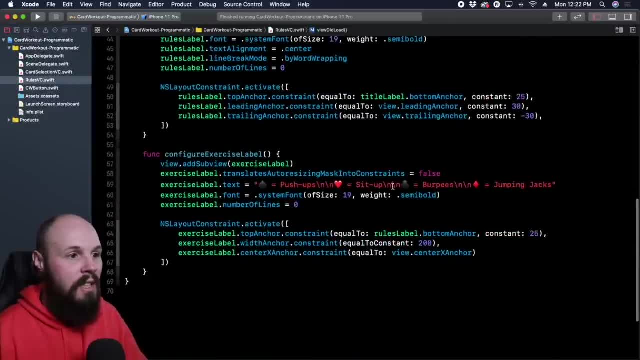 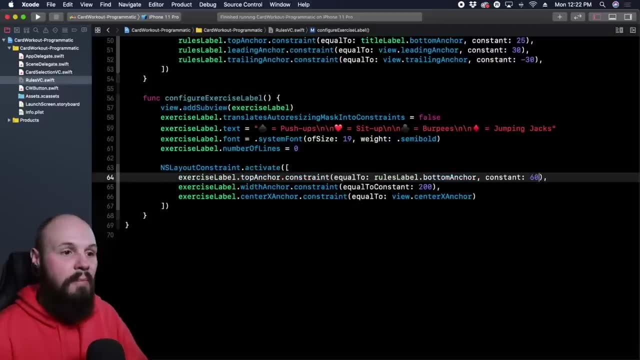 That was actually more So. I believe it was like 50 or 60. So again, exercise label, rulesbottom anchor. Let's change this Instead of 25, let's change this to 60.. And again, this is also the power. 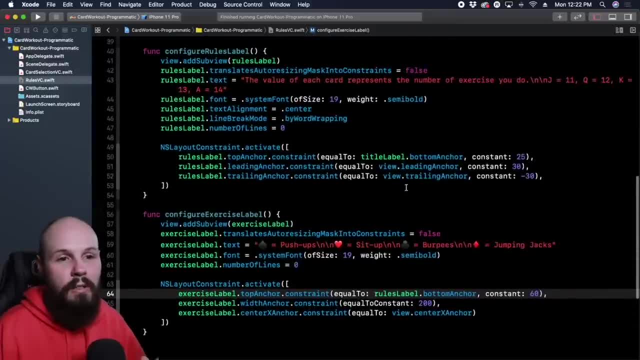 of doing your UI programmatically right For me to simply change a constraint. I can like, toy around with these and change them real quick to dial it in, Whereas on the storyboard it's kind of a pain. right, You gotta click on the object. go to the ruler tab. 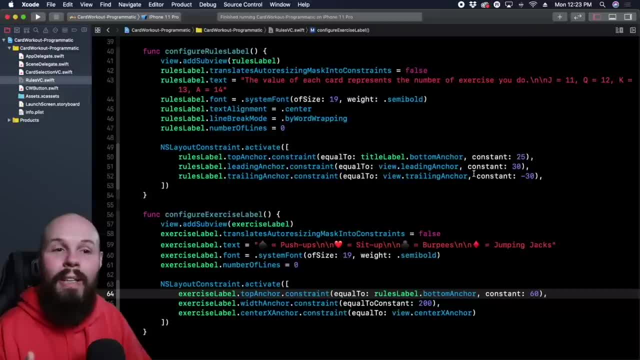 find the constraint edit the thing right. This is, you can really quickly edit your UI just by changing some numbers around. when you do it in code, Of course, the initial setup takes longer, but I view it as like an investment. 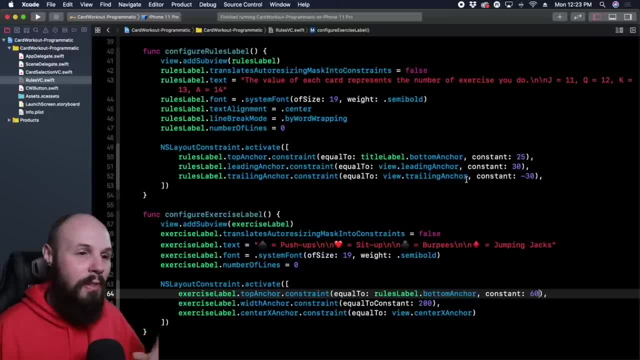 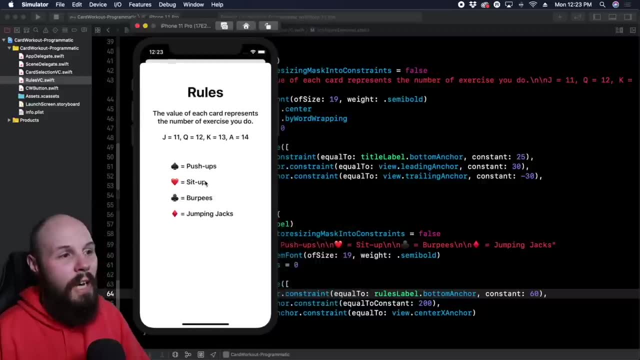 Like, yes, it takes longer to set up, but making changes, making additions, so much faster in my opinion. So now let's run this again And we're going to see our rules. Now we've moved that down a little bit. 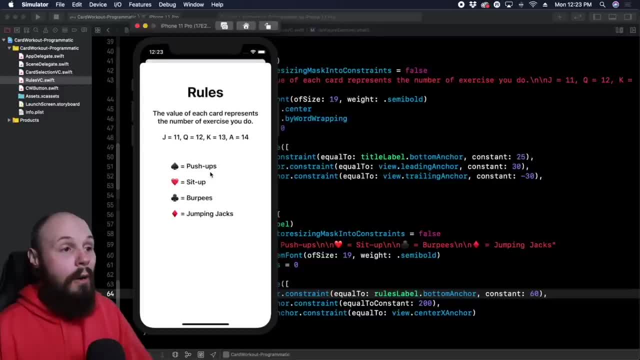 Okay, good to go. So, as you can see, that laid out our rule sheet. but let's take a look at this. Remember, in storyboard there was no code at all. We just laid all that out on the storyboard. Now, when we stop this like 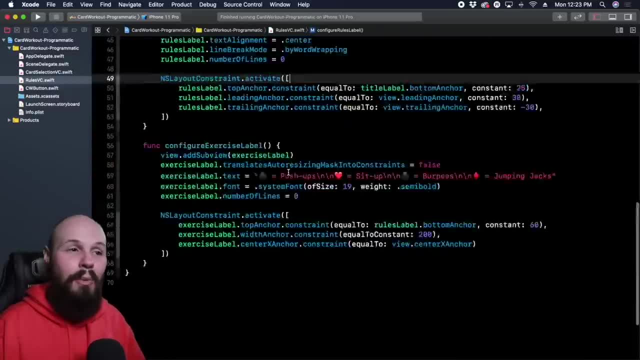 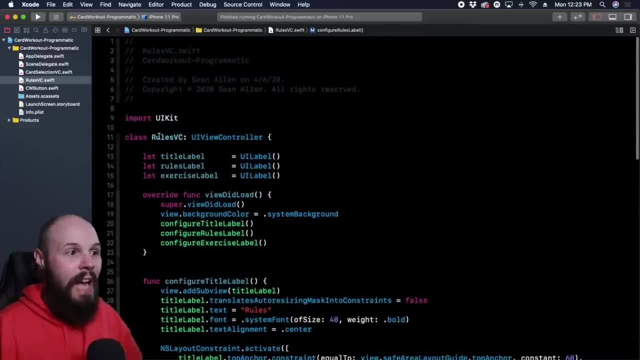 let's look at all the code we had to do just to replicate that simple screen, which we did relatively quickly and simply just in storyboard Like. remember, on the storyboard project we didn't even have a view controller called rules VC, We didn't need one. 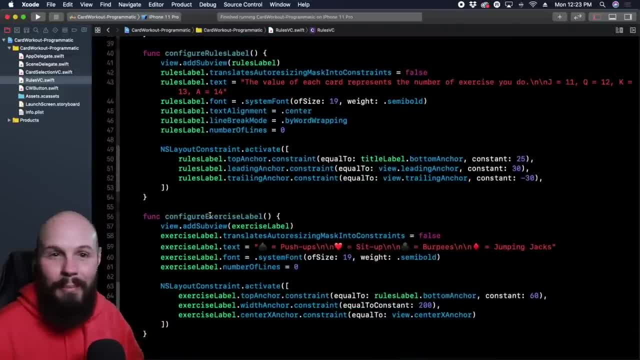 So again, pros and cons, again. that's why it's a debate, Like: sometimes storyboard is quicker and easier, Sometimes code is better. So, like I said, that's why a lot of people disagree and that's why it's a pretty subjective. 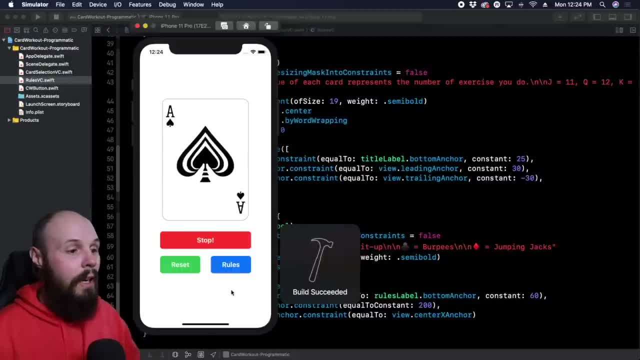 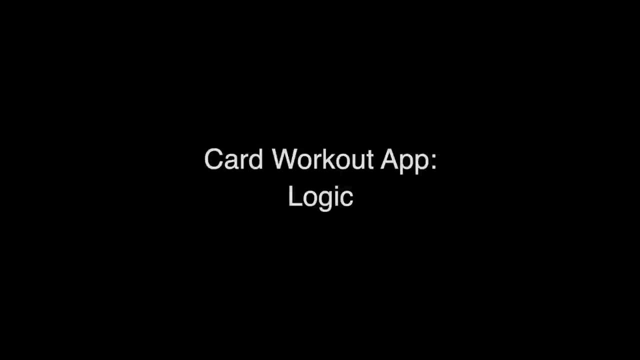 but we have our rule sheet. Let's run it real quick to leave it up there. That is laid out. All we have to do now is start doing the logic of the app. Let's go Again. here we are right where we left off. 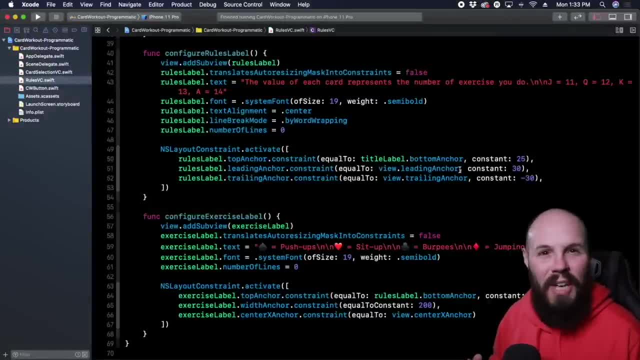 Now all the programmatic UI. well, 99% of it is done. We still gotta add some button targets to the other buttons, but essentially, at this point all you have to do is add the logic that we did in our storyboard. 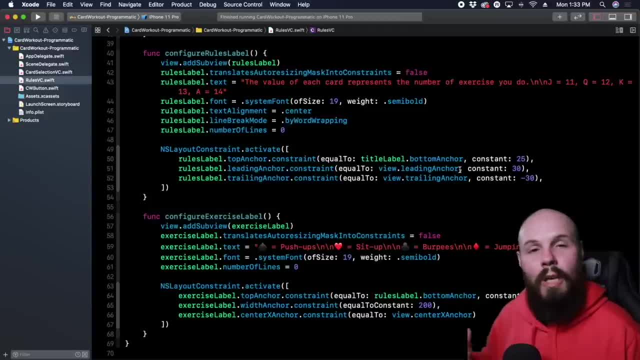 So here's a little challenge for you. If you'd like try to finish this project on your own before watching this video, getting it up and running in the programmatic project, Okay, pause it now. Sure, pause done. All right, if you did that, hope that went well. 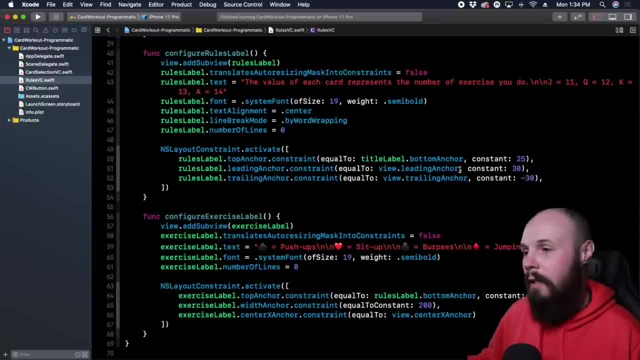 If not, this was just like two seconds ago. Now it's weird. Anyway, let's move on. We're gonna do this together here. We're gonna finish up this project. So let's run this just to get a state of the union real quick. 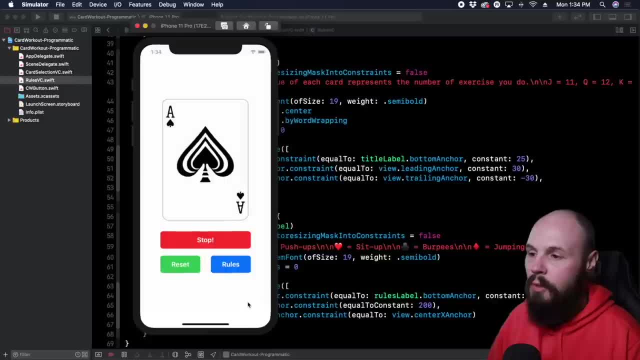 Where are we at? So when we tap rules, we can see our rule sheet. that's working: Stop and reset. So we have to implement our timer and then the array of all the card images so that it can cycle through And then stop it with the buttons. 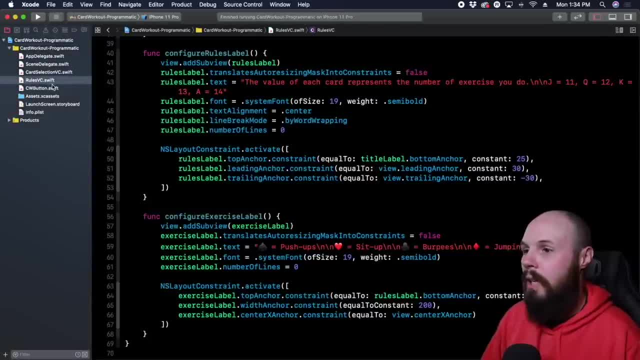 and reset it with the buttons. So first thing I'm going to do is create our card struct. Well, I'm gonna rename it because that was a horrible, horrible name. Naming is hard, Anyway. so in the folder, do Command N. 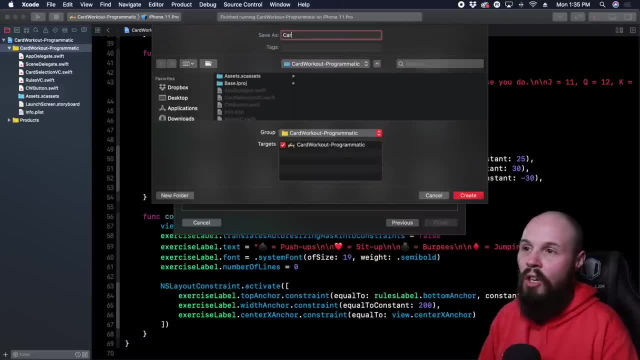 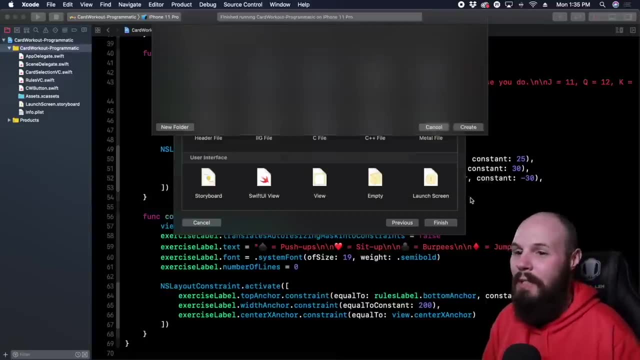 It's new Swift file Hit next. I'm gonna call this card deck. That's what I should have called it last time. This is gonna have card deck dot all values. Like I said, naming can be difficult, So that's called card deck. import UI kit. 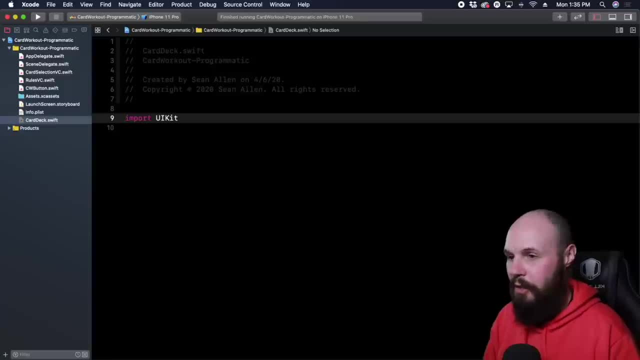 And actually you know what? I'm just gonna copy and paste this from the previous project. I suggest you do the same. I'm not typing this out again, So here, return, paste. This is the card from the storyboard project. 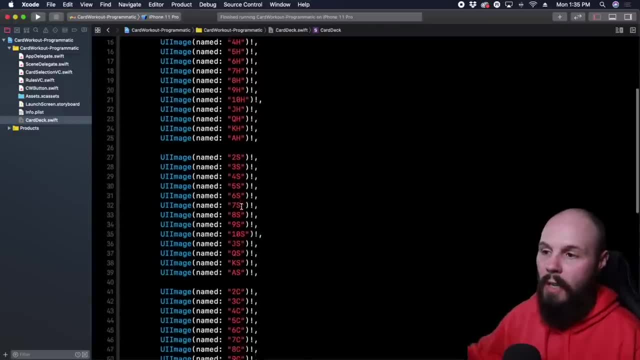 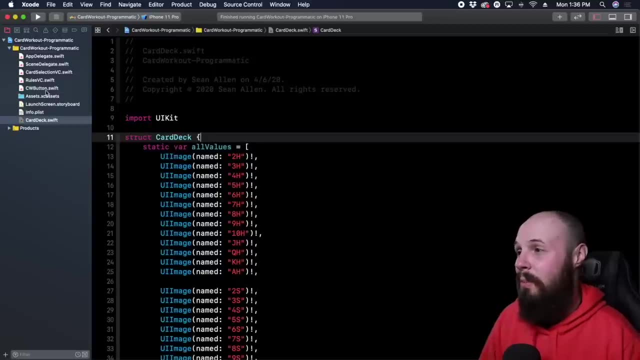 Again, we're gonna name this card deck. So here is the array. Again, we went over this, typed it all out last video. We're gonna save some time in this video because it's the same And a lot of this is the same as well. 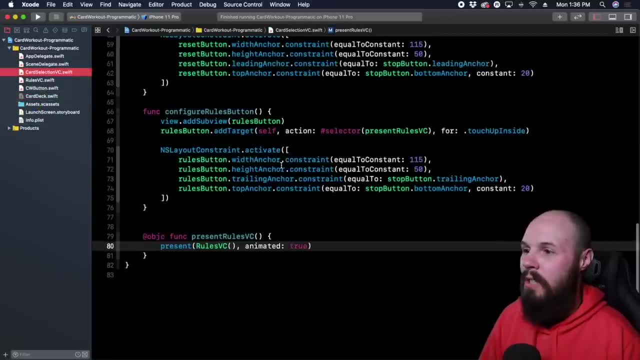 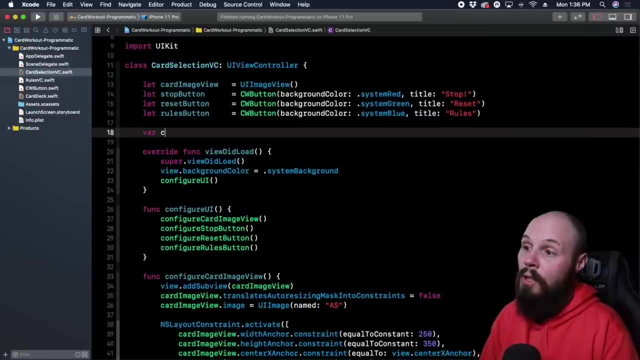 So back to our- we'll move this up a little bit too- Back to our card selection VC, Up at the top part of our variables. here we need a variable, an array called cards, which is an array of type UI image. 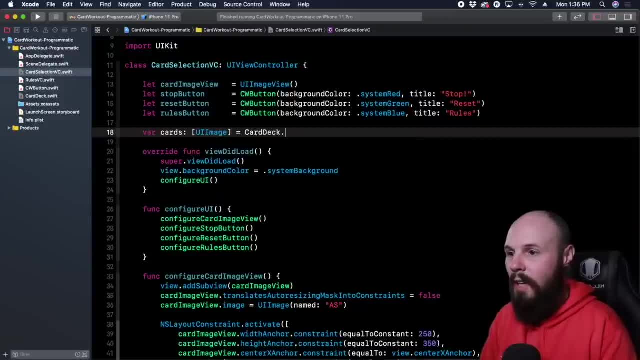 And that is going to equal card deck All values. right, What we had there- And to be honest with you, we don't need to declare the type here, We can just do cards- equals card deckall values, If you want, right. 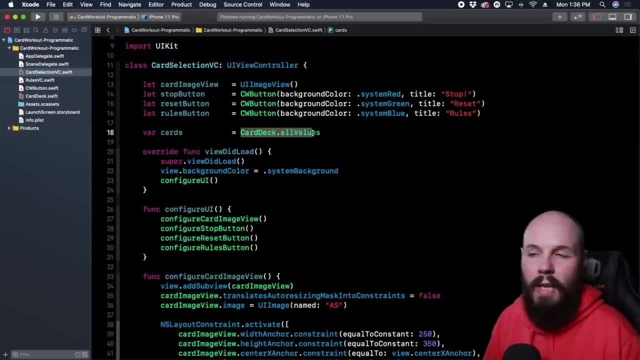 Cause you don't just looking at this. you don't know what card deckall values is Like. what is that an array of You know. if you've built the app, you know what it is, but you understand how this could be confusing. 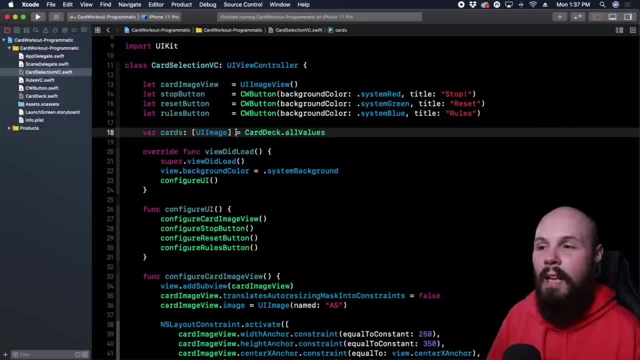 So, leaving the type declaration. there is a way that you can easily see like: oh okay, This is my array of UI images that I'm using, So if you think that makes a more readable code, leave it there If you want it to be a little more clean. 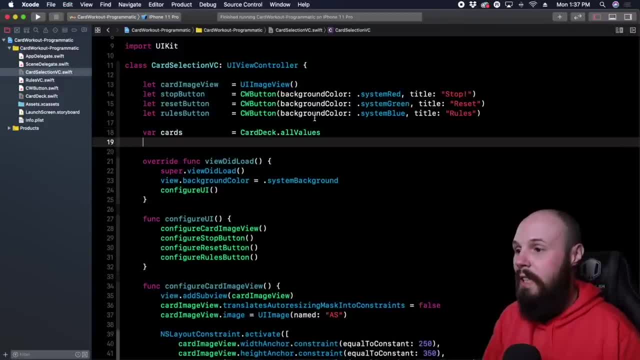 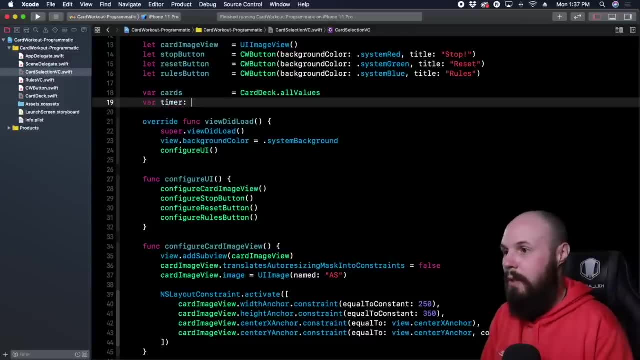 just do that And I'm going to line up my equal signs. The other thing we're going to need is our timer, So of our again, this is just repeating what we did before, Our timer of type timer and exclamation point. 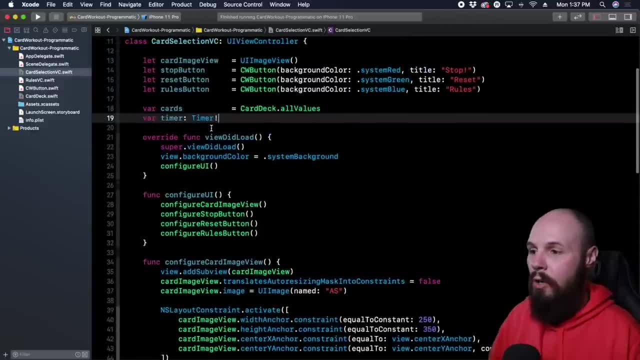 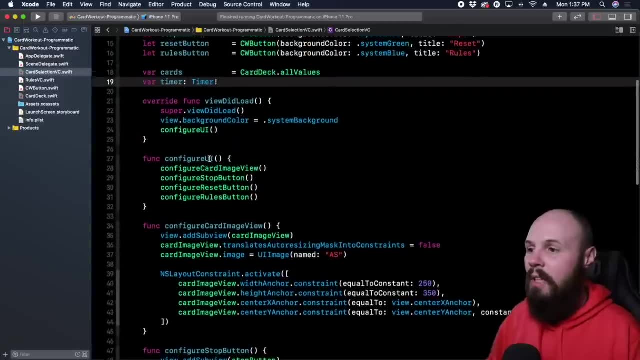 And we need to start our timer down here. Now the way I like to lay out my code. right, You see, we have all this UI code. I like to push that towards the bottom. You know, I like the logic and the functionality. 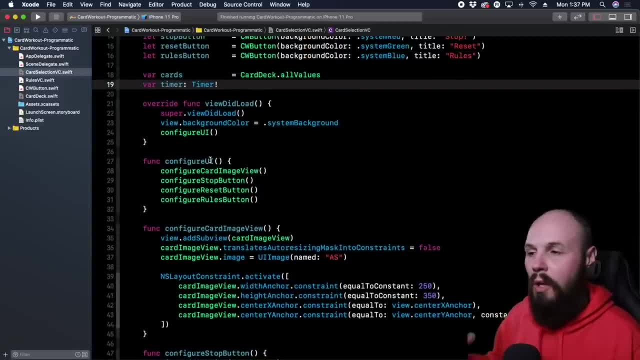 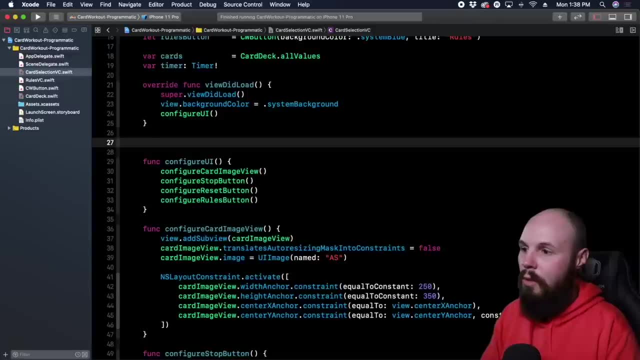 of my view controller to be up top, Cause that's usually what you work with a lot, And then if I need to change my UI, I know I go to the bottom, So I'm going to start putting all these other functions up here towards the top. 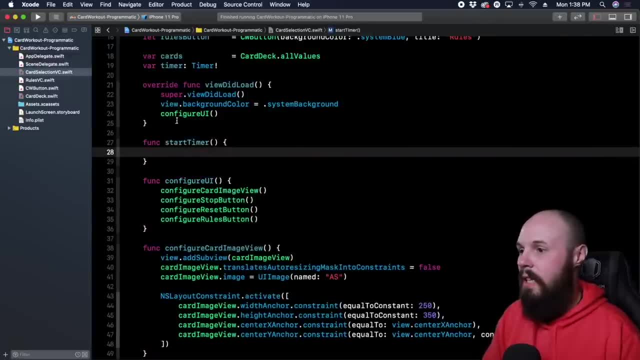 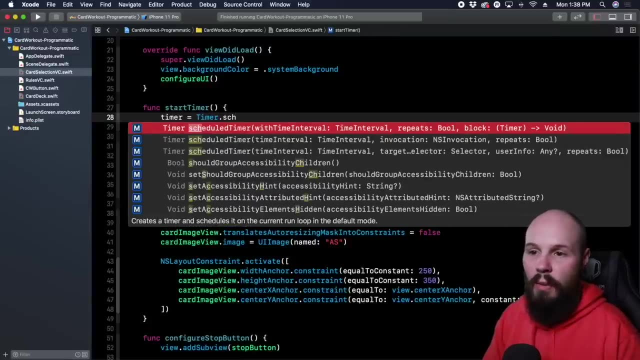 So we need funk: start timer And then remember we did a timer equals and then we initialized a timer dot scheduled timer And we did the one with the selector. So remember time interval 0.1.. Again, this is all review. 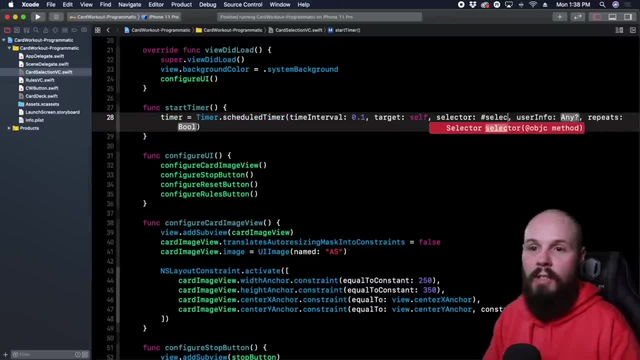 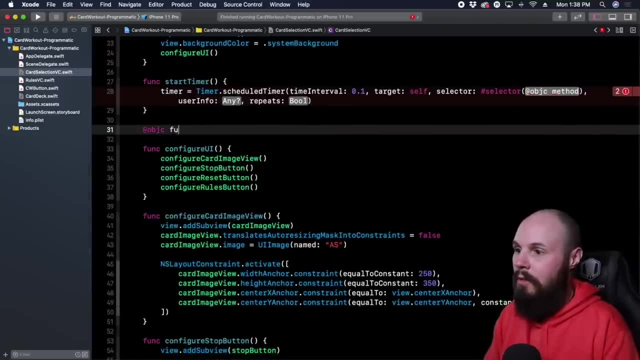 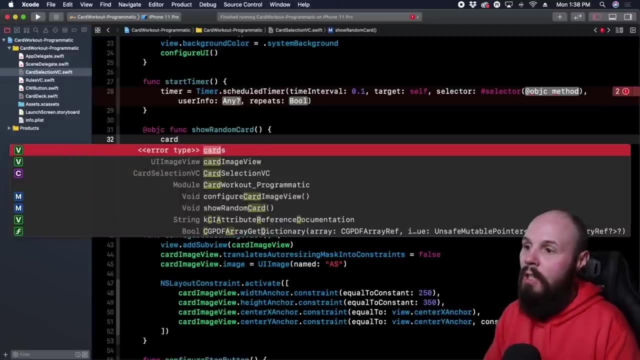 Target self selector, Hashtag selector. Now we need that at OBJC method. So we want to fire off show random card. So at OBJC funk, show random card. And then remember in the show random card function it was card image view dot image. 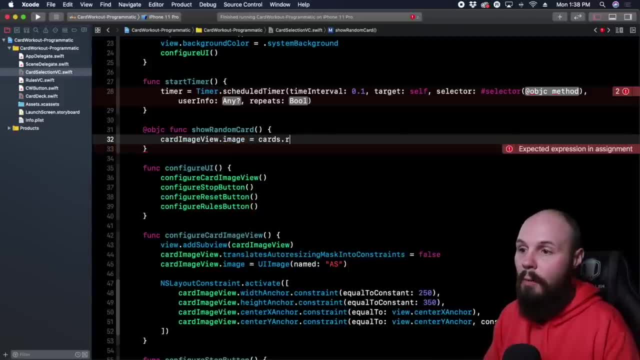 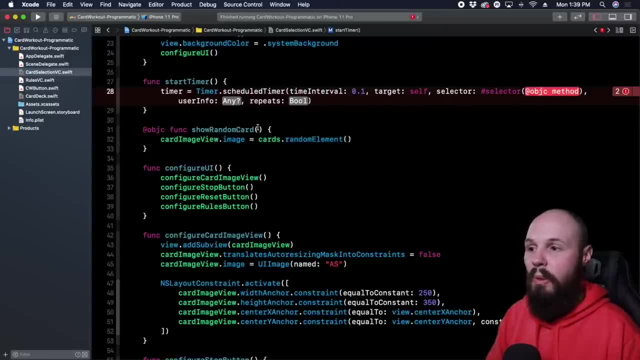 equals cards are: array dot, random element. There we go, So let's finish up this function. signature here Again. hashtag selector: We want to pass in Show random card Again. this is exactly what we did in the previous project. User is nil. 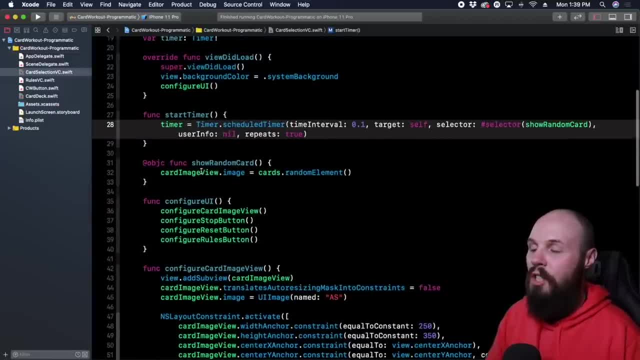 Repeat True. So now that timer fires off, we're going to change that. Let's test it Again. you always want to be testing your code along the way. I bet I didn't call start timer Again. it's going to happen to you all the time. 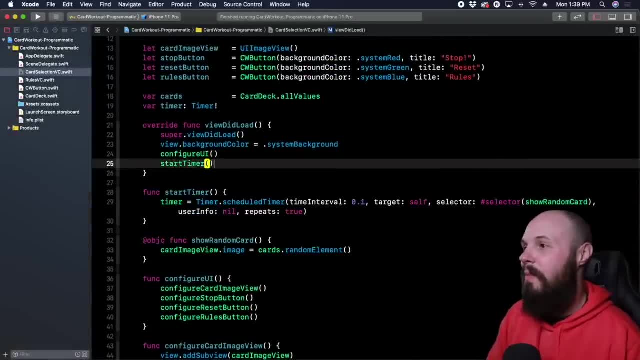 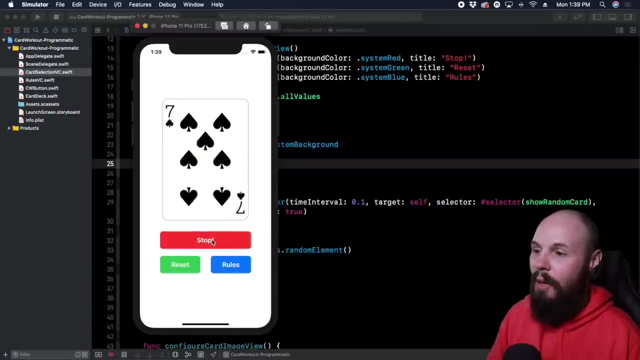 So, after configure UI call start timer, Now run it Again. silly mistakes all the time. There you go. Now hit stop. We don't have the stop button set up, OK, so that's what we got to do. But we know our timer is working as expected. 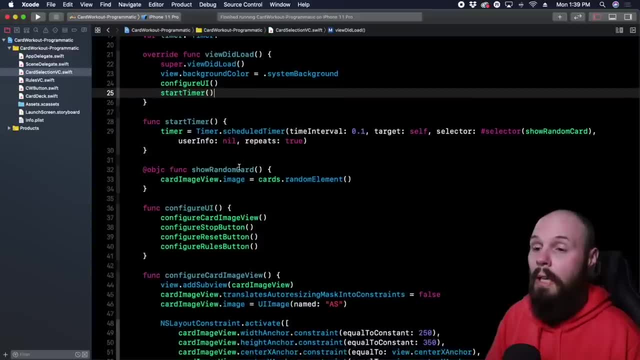 So again, piece by piece. So now we need to handle the stop and restart button. So we need to put action or targets on those buttons. Sometimes I call them actions based on the storyboard. It's an IB action, But we need to add a target to the buttons. 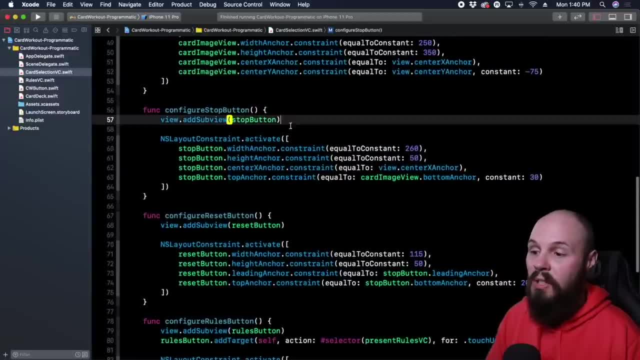 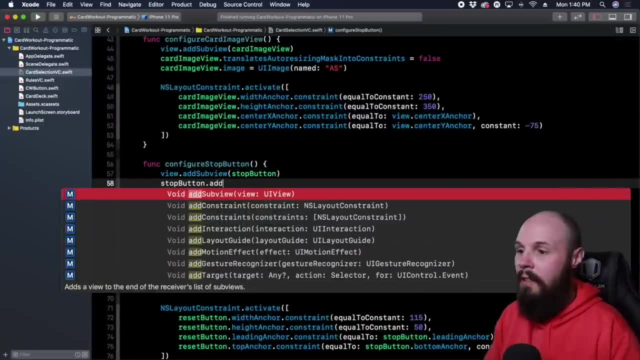 So our stop button here: configure stop button just like we did with the rules button down here, where we had rules button dot add target. Here's how we add the target here: Stop button dot add Target. Here we go. Target is self action. 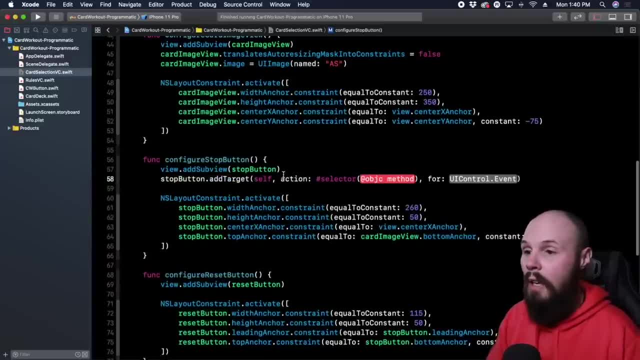 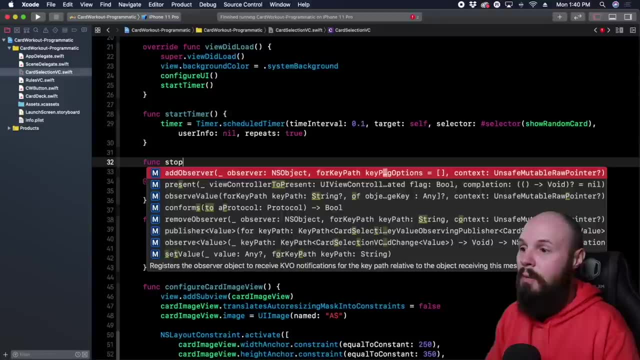 Hashtag selector. Again, here's where we need to pass in an OBJC method. What we want to do is we want to stop the timer. So, again, we have a function called start timer, func, stop timer. except this function needs to be at OBJC. 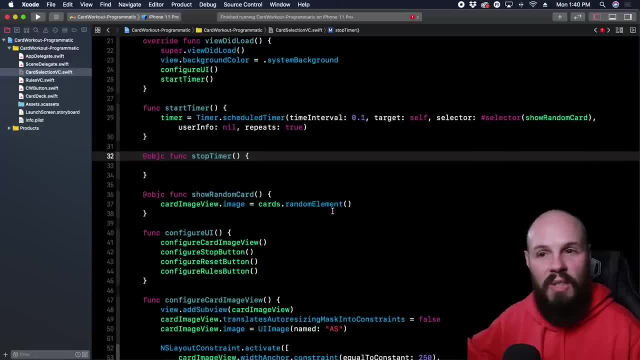 Remember, when we're using these hashtag selectors, we're interacting with objective C Again at a lower level, not at our high level here. So that's why we have to declare this as an at OBJC method. So stop timer. 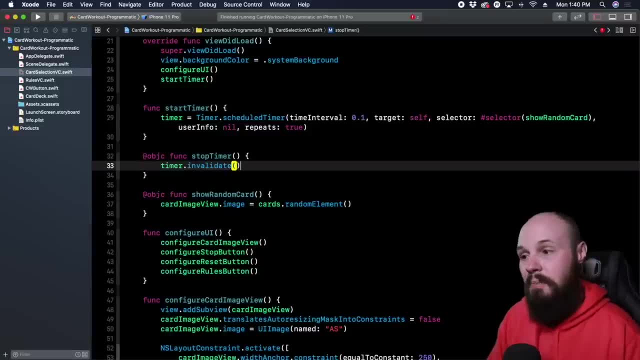 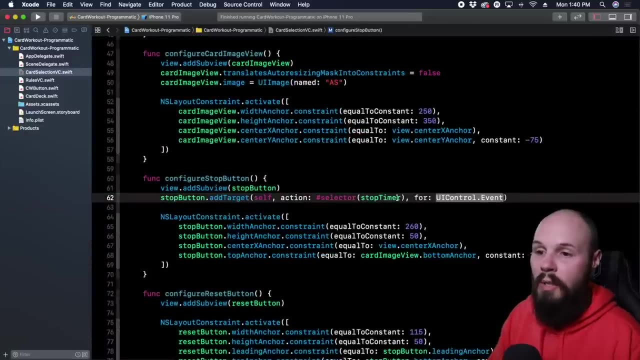 See, if you remember, it was just timer dot invalidate- Again same exact thing. So for the stop button, we want to pass in stop timer that we just created up there, and for dot touch up inside. That's the default for the button. 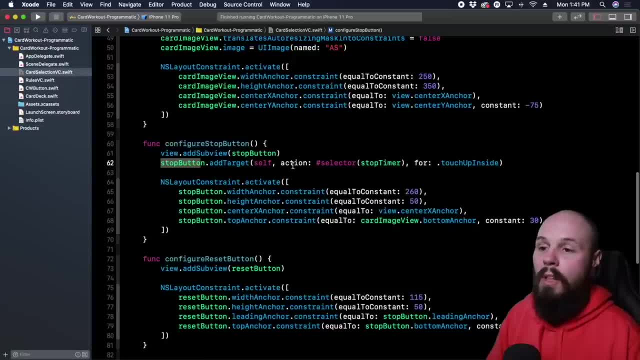 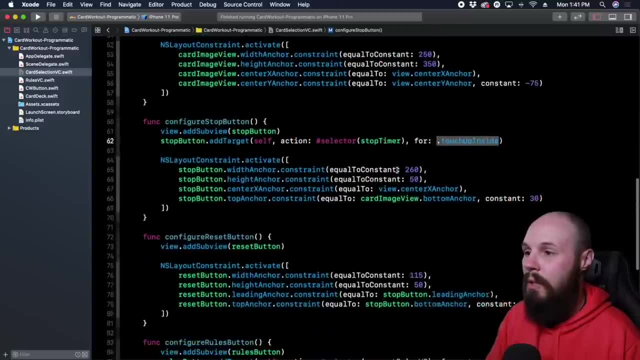 So what we did here? we added a target to the stop button that fires off start timer when the touch up inside, which is just a normal press. So now we need to handle the reset button. So here in the configure reset function, do reset. 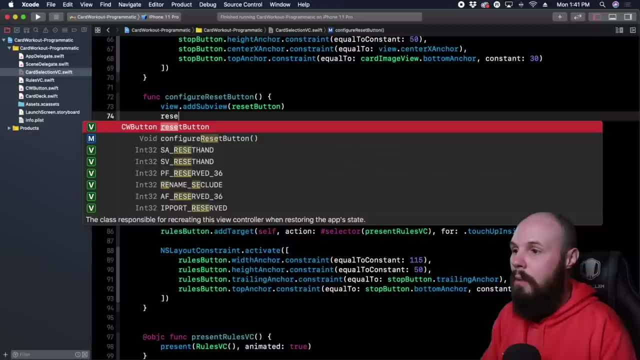 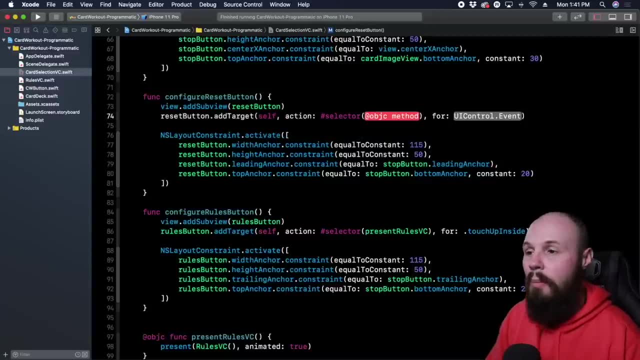 So here in the configure reset function, do reset. So here in the configure reset function, do reset Button dot. add target self for the controller Hashtag selector. Again, we need another at OBJC method. This method is going to stop the timer and then restart it. 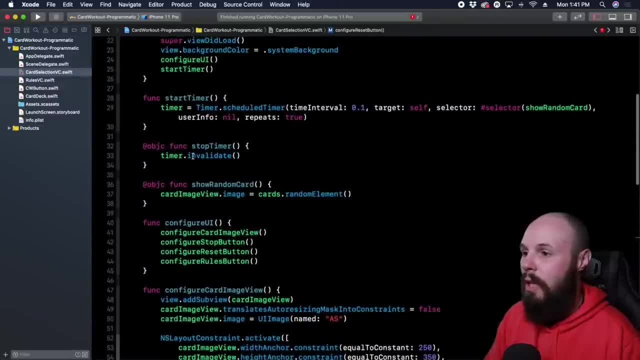 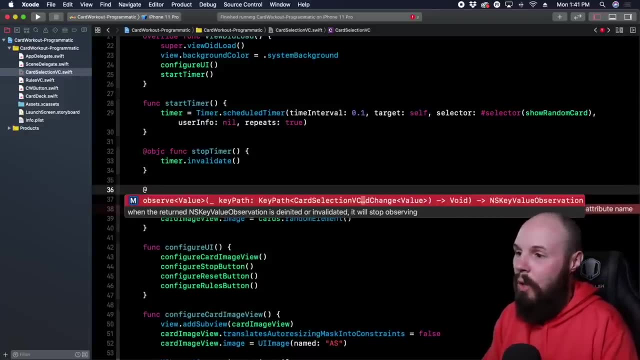 So let's create a method here, right below stop timer, And again I'm breaking these out. You could write some clever functions that combine these, but I'm just writing these out so you can see the steps of what is actually going on. 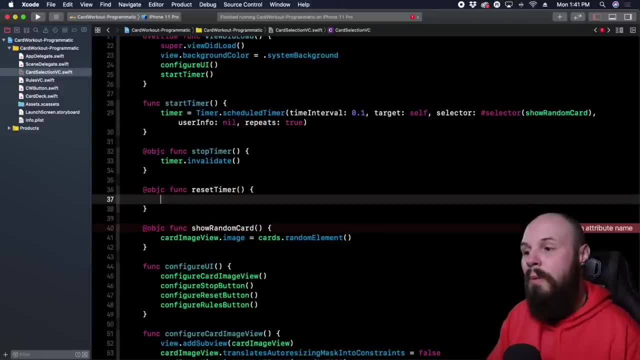 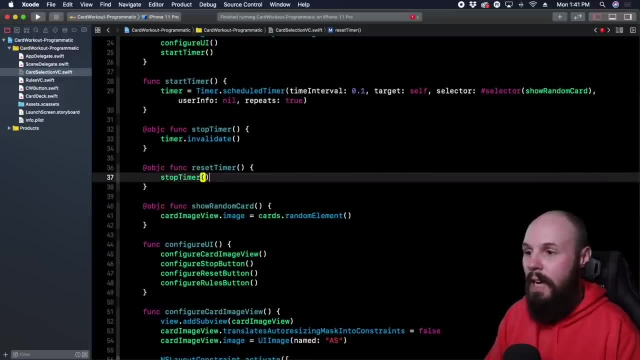 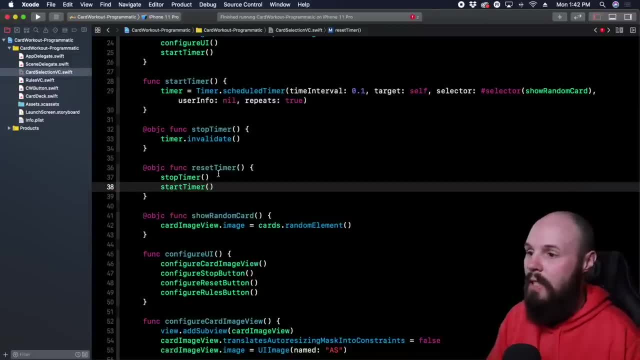 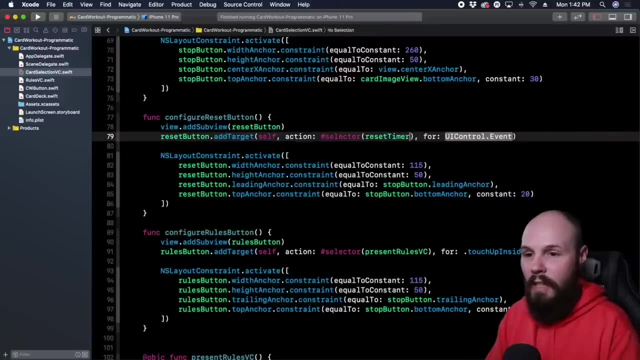 So do start timer. There you go. So that is our reset timer function, And down here in the at OBJC method of the reset button we can do reset timer. And then again- that is also for dot touch up inside, which again is the default- tap the normal button, tap. 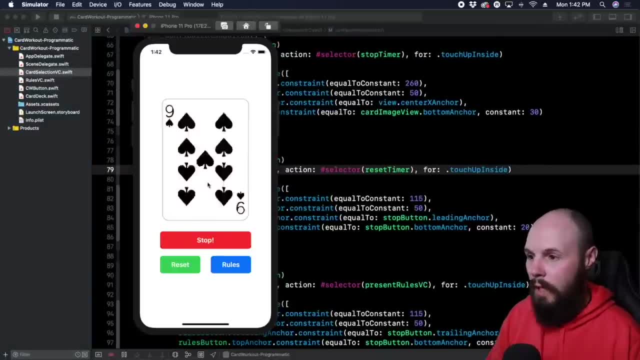 So our buttons should be working. now Let's run it and test it out. Okay, It's cycling through. stop, Cool, Stop works. Does reset work? Hit reset, Reset worked. great, Hit reset, again Cool, It's stopping and restarting that timer. 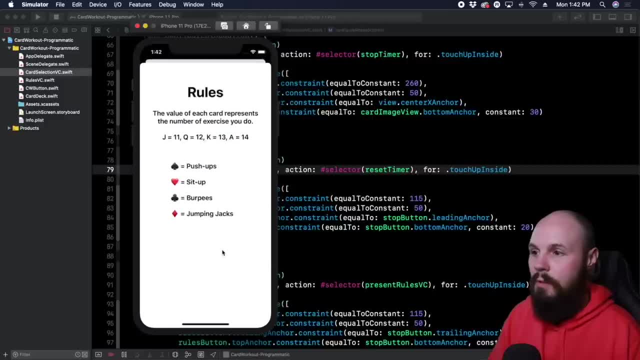 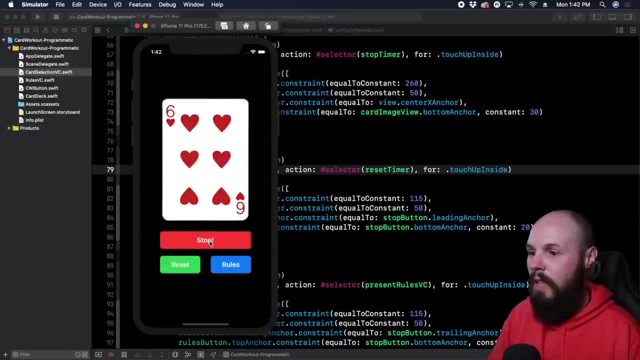 Stop Reset Cool. Stop Rules. Nice, Let's do the old command. shift A for dark mode: Looks good, Reset Looking good in dark mode, Stop Rules, Cool. Our app is up and running 100% programmatic. 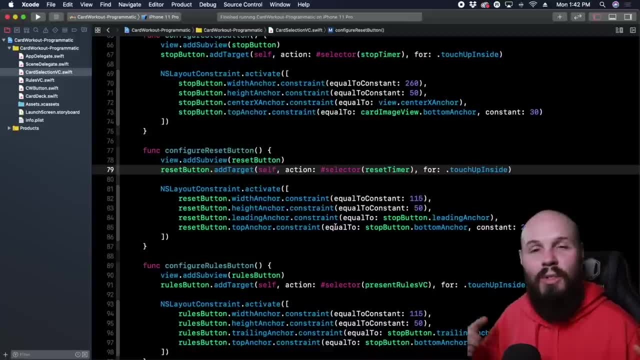 So now that you've had a taste of both worlds, you can start forming your own opinions and what you like more. Here's what I always recommend For those that are just learning. I find programmatic is the better way to learn because you start seeing what's going on. 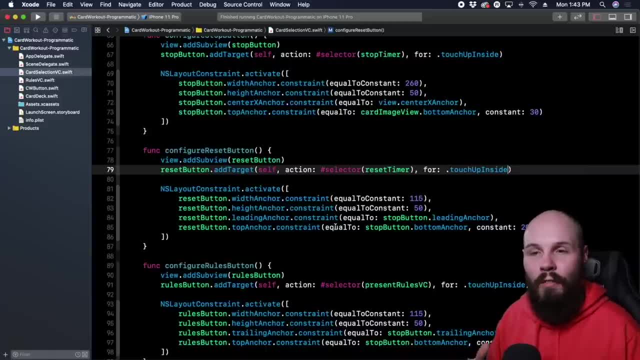 under the hood, so to speak. right, It's easy on the storyboard for it to be like magic, Like I don't know. the storyboard handles it, but you don't really know what's going on. However, when you're laying out all your constraints, 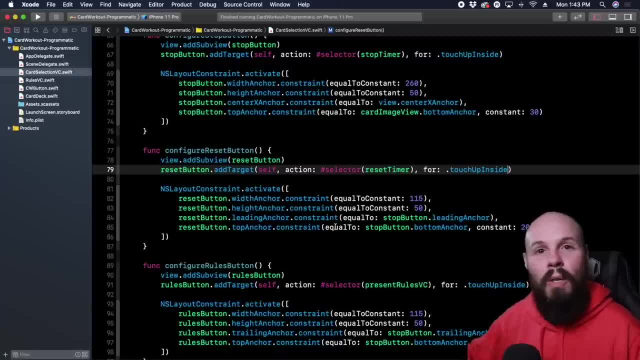 in code. you're adding targets to the button. you can see what's going on under the hood And I think you learn the fundamentals a lot better, a lot better when you do programmatic. Now, once you've learned programmatic and you're more experienced and you can do both no problem. 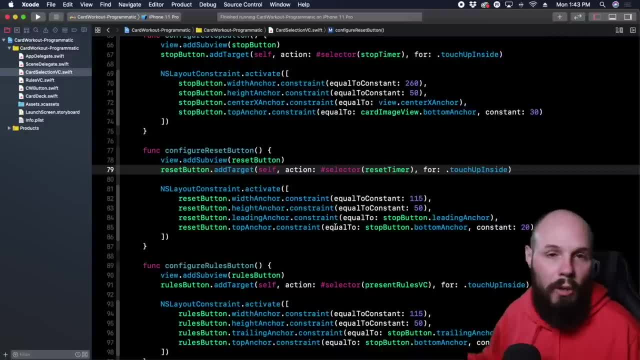 That's when I at least what I do. I've shifted towards what I call using the right tool for the right job, And, again, a lot of my projects are a mix of both programmatic UI and code, And the perfect example is that rule sheet. 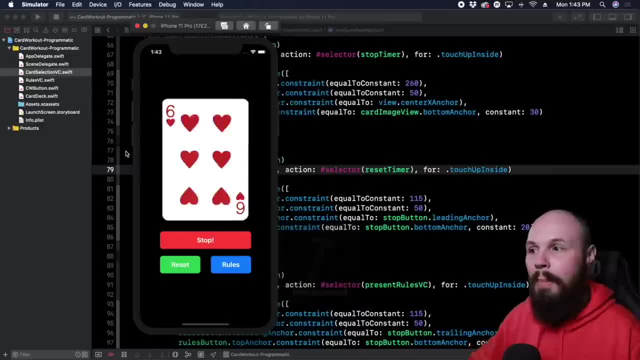 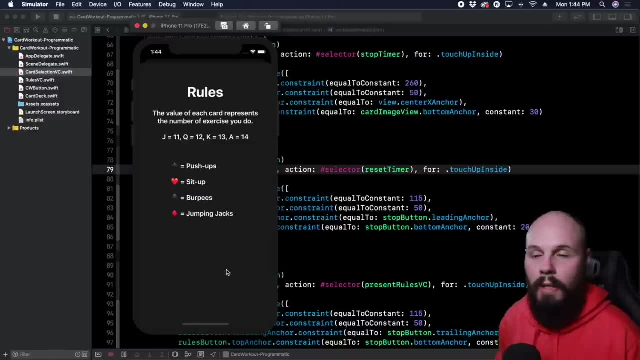 Let's run it here. So if I was building this project for real and this was like a real app, I was building- like I said, I usually do- a hybrid of storyboard and UI, So the rule sheet would absolutely 100% be done on storyboard. 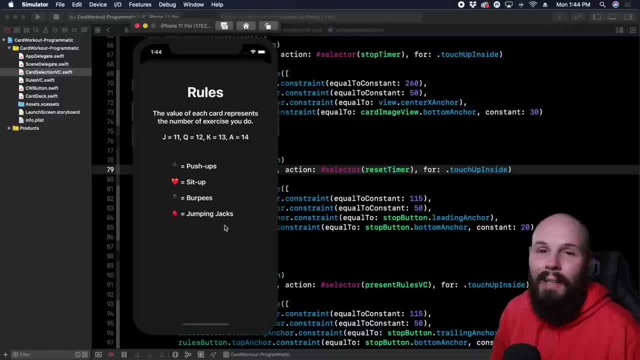 Like I'd have no code for that right Cause. again, that's the super simple layout, You don't need code. And this screen I don't know. it depends on what else would be on the screen, I guess the only hard and fast one I know for sure. 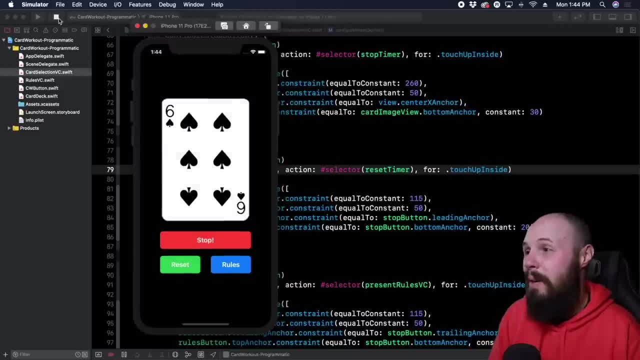 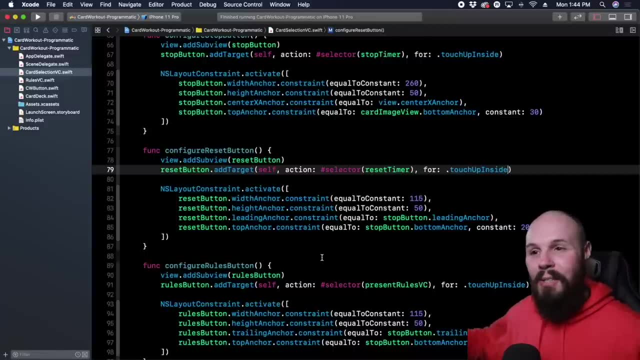 I would be doing this 100% storyboard, But again, those are just my opinions and how I like to program The point of me showing you both, like I've said 35 times by now, start forming your own opinion And that's a corollary for just programming in general. 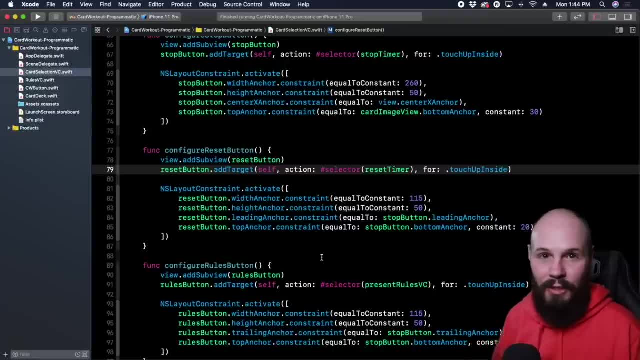 Like I've said before, it is a very opinionated field. You're going to see things online. People are like: no, this is wrong, This is the worst way to do it, This is bad, And you'll see somebody else saying no, no, 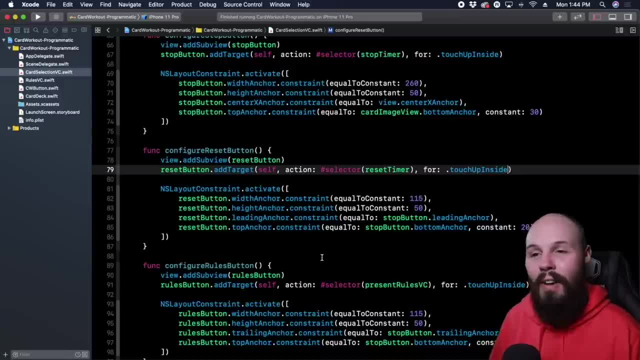 that's the best way. Again, very opinionated. I find the best way to deal with that is to educate yourself, try the methods and form your own opinion, right, Don't? I guess the moral of my little rant here? don't just blindly listen to people on the internet. 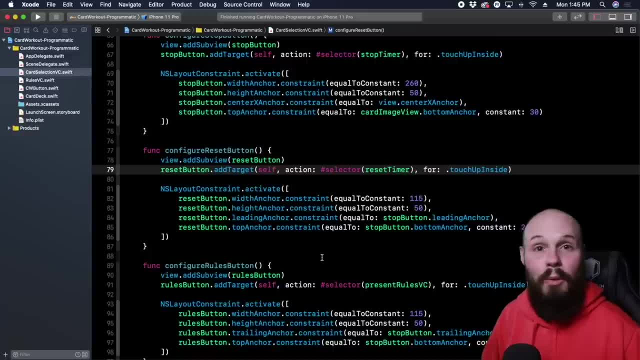 Cause. again, if you listen to one person, you'll find another, experienced, reputable dev that will think the exact opposite. So that's why it's a tricky field, Very subjective, but again, educate yourself, form your own opinions. We are done with the card app. 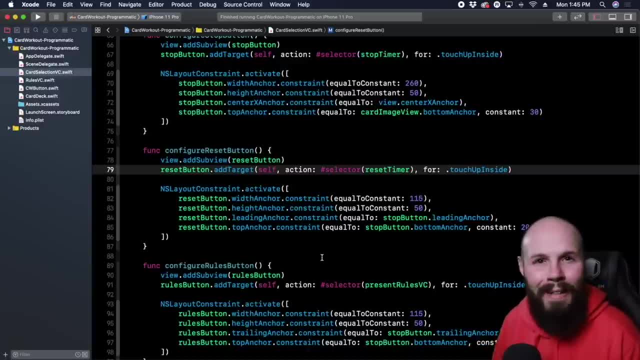 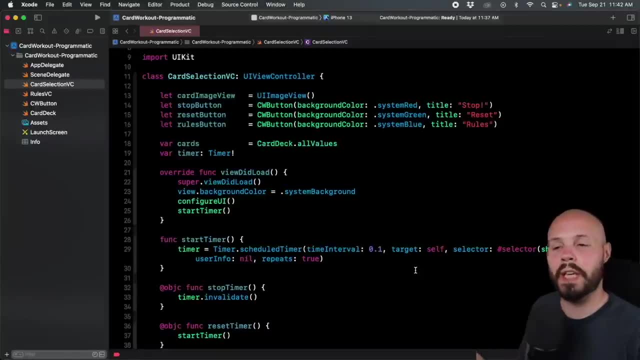 Cool Again, you saw it both ways. Now we're going to move on to the old, the new hotness, Swift UI. In the last video I showed you how to use the new button configurations in Storyboard. I also gave the overview of what these buttons are. 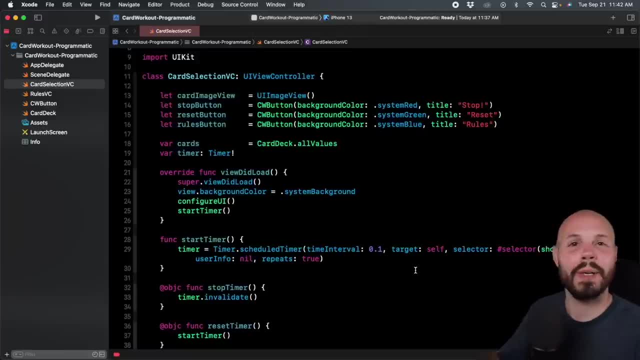 showed you the WWDC videos, So if you skip that one, I'd recommend going back and at least checking out the beginning, where I explain everything, because in this video we're going to do the same thing we did in that video. However, everything will be done via code. 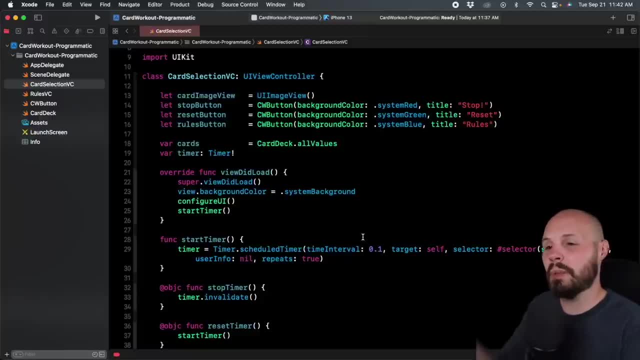 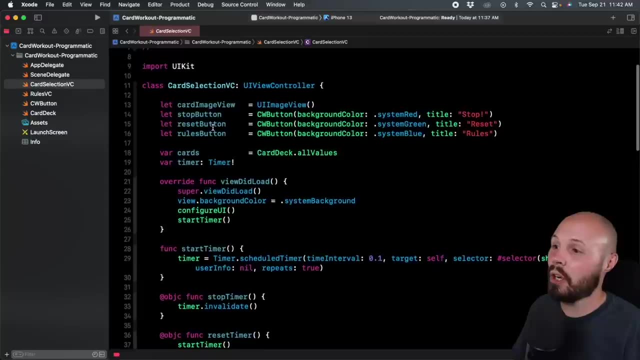 and not Storyboard. Again, keeping with the thought process of doing it both ways, And then you deciding if you like Storyboard better or code better, or at least you just know how to do it both ways. Anyway, here we are in the card selection VC. 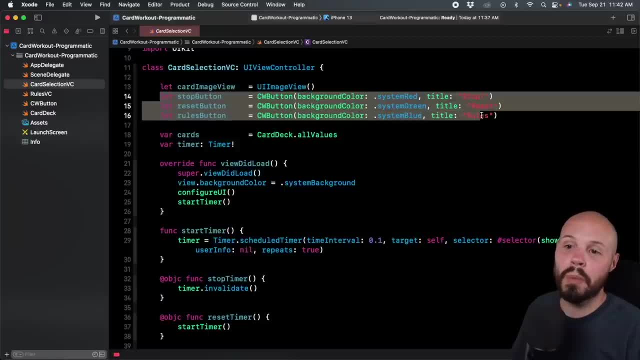 So, as you can see, we are initializing three CW buttons here. right Again, this is the old code that we had. By the way, I didn't mention that This is the existing card workout project in Programmatic UI. This is the existing card workout project in Programmatic UI. 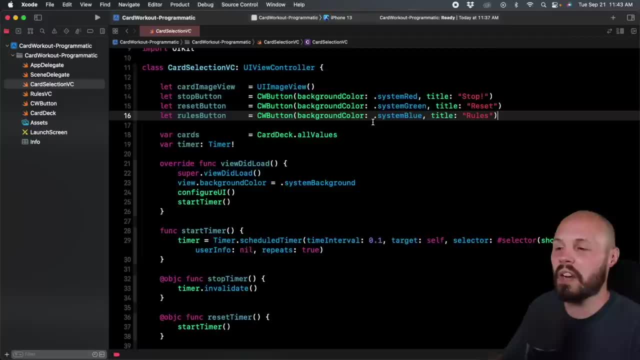 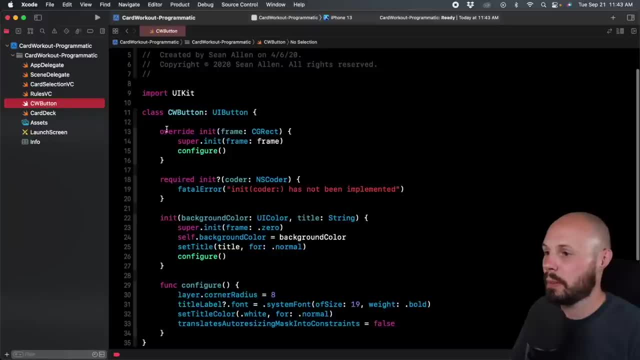 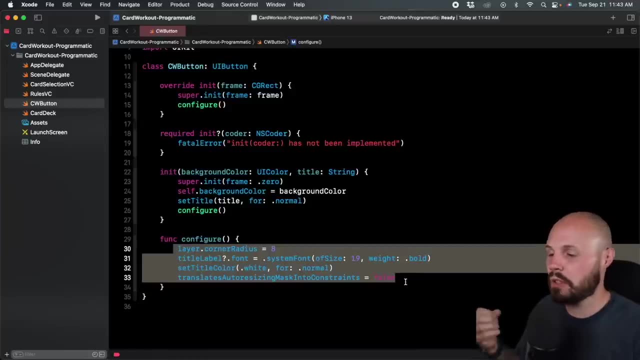 in this CW button class which we created down here. if you remember right, This is our custom button. So, essentially, what we're going to do is get rid of this configure method, because we're not configuring it ourselves. We're using the U button configuration. 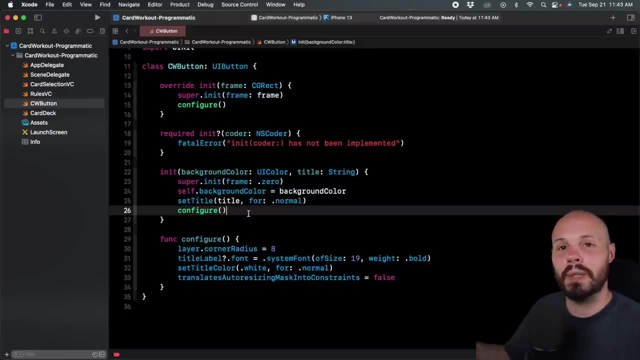 and all that will be done in the initializer. So that's the big picture of what we're going to do. Now let's start coding it up. So the first thing we want to do, let's just make some space. I'm going to be like deleting. 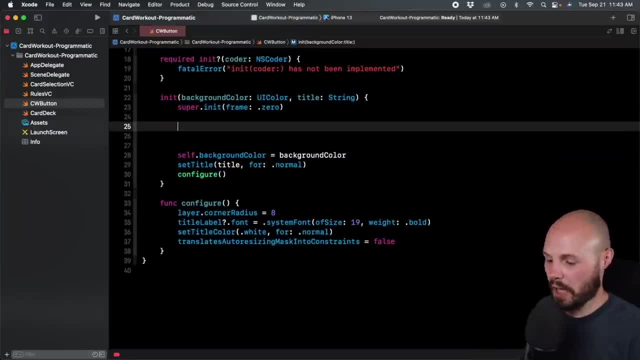 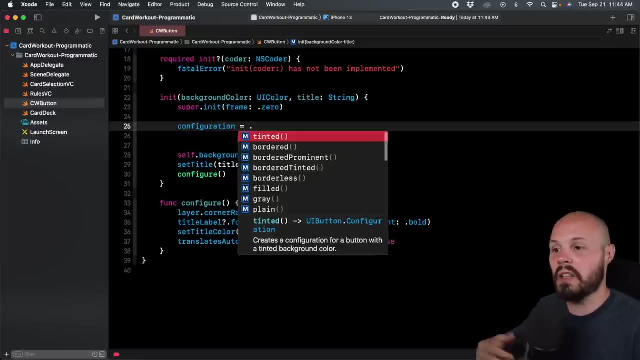 and commenting stuff out as we go, But the first thing we want to do in our initializer is decide which configuration it is. So we'll say configuration equals and I'll do dot. And you can see these are the styles right, Dot, tinted. 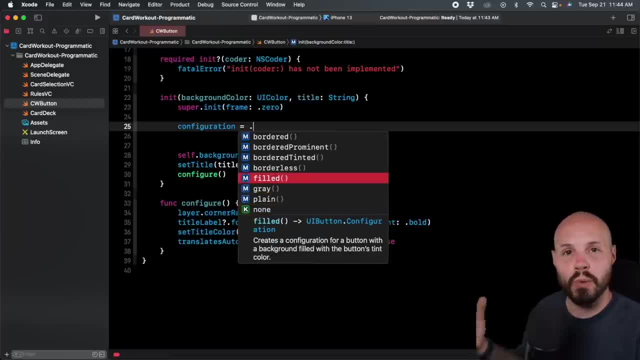 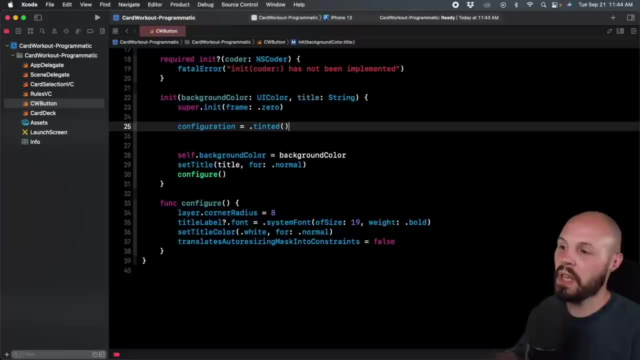 Well, there's more styles here: Filled gray, plain, right. That's what we worked with in storyboard. I showcased what they are in the last video, So we'll just skip right to what we're doing, And that is the tinted configuration. 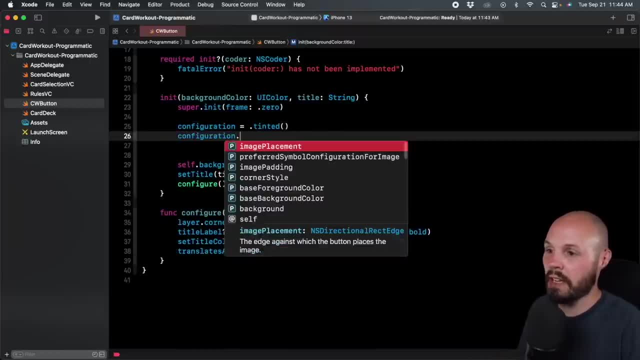 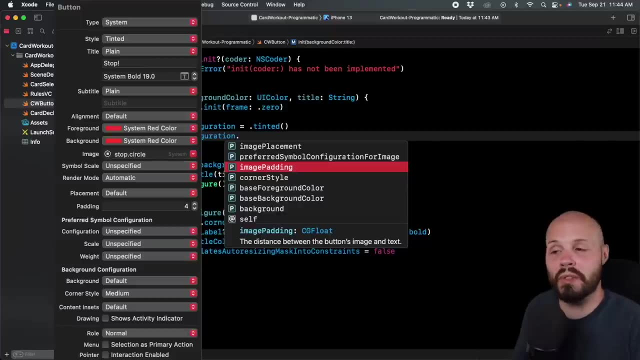 So now here we're going to do, you know, configuration dot, and then you're going to see all the properties we got in the storyboard. I'll put a little screenshot of the right pane that we were working with in the last video. 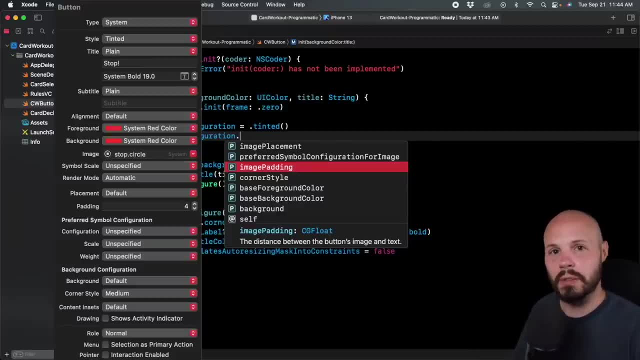 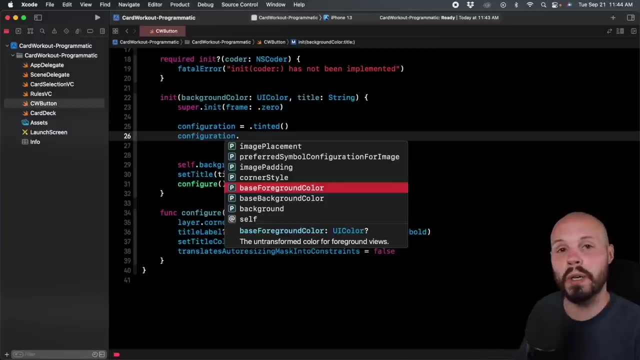 Basically all that stuff is the same just now in code, So we're going to recreate what we did last time in code. So let's handle our background color and our foreground color first. Remember the foreground color is the text And because we're doing tinted, 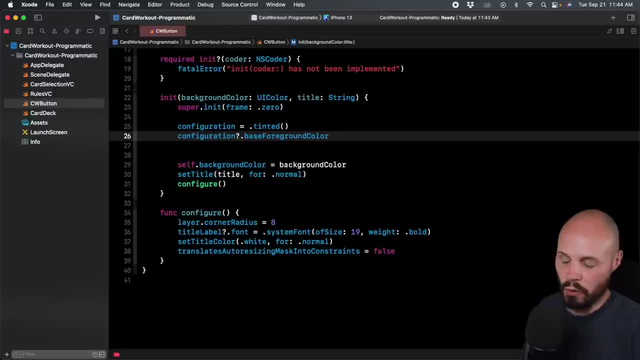 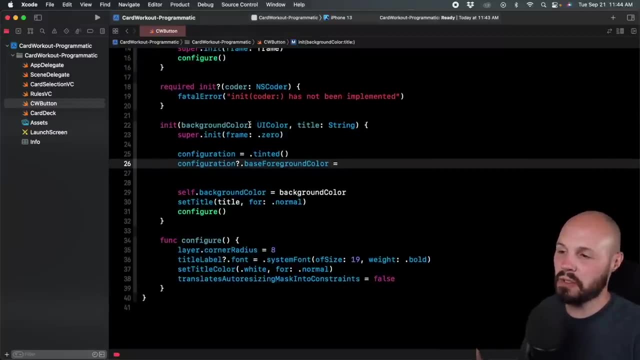 these are going to be the same color, So we want to set our base foreground color equal. to remember this initializer, we're passing in the background color. Well, because we're switching to tinted buttons, background color isn't really accurate, right. 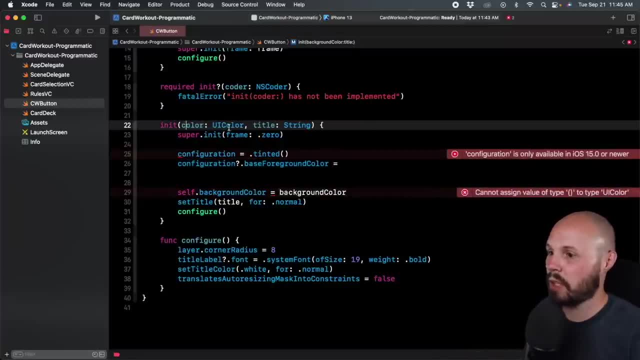 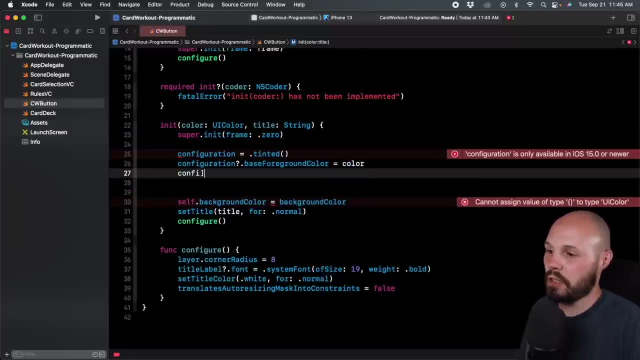 We just want to call this color right. It's to be clear here. So color is what we're going to pass in, And I want to make this equal to color. And then the same thing down here: configuration: dot base background: color equals color. 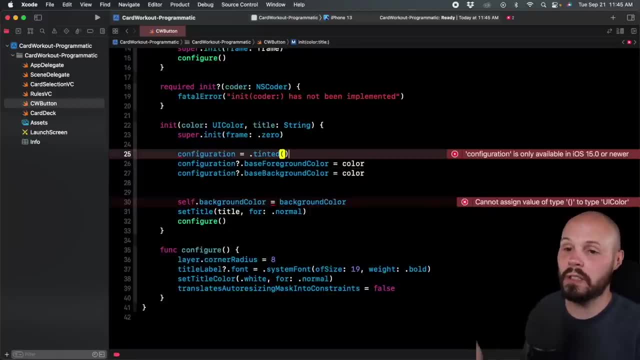 Because, again remember, the background and the foreground are the same color in our tinted configuration. Ah, good catch. here, Configuration is only available in iOS 15 or newer. Well, this is the what's new in iOS 15 section, but why are we getting that error? That's because I pulled up the old project- maybe the one that you're pulling up as well- And that supports iOS 13.. So in our card workout target here, right, iOS deployment target, let's change that to iOS 15 and then targets: a card workout. 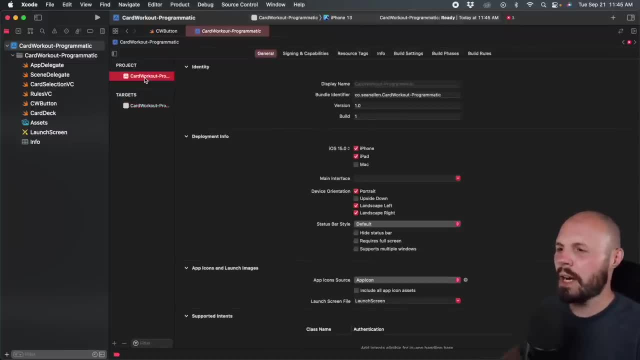 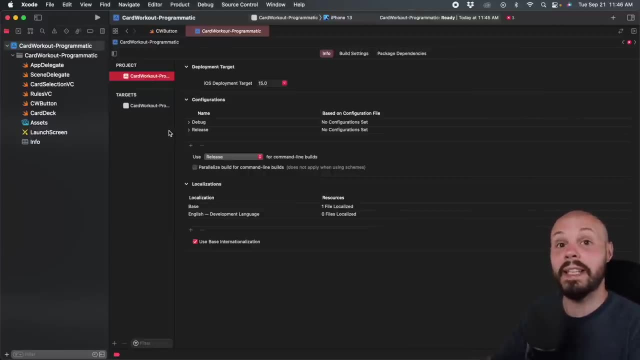 when you do, oh, that is already targeting iOS 15.. So I don't think I did that in the storyboard version, because I think maybe I had done that off camera. So my apologies if there was confusion there. I'll be sure to make a note in the edit of that video. 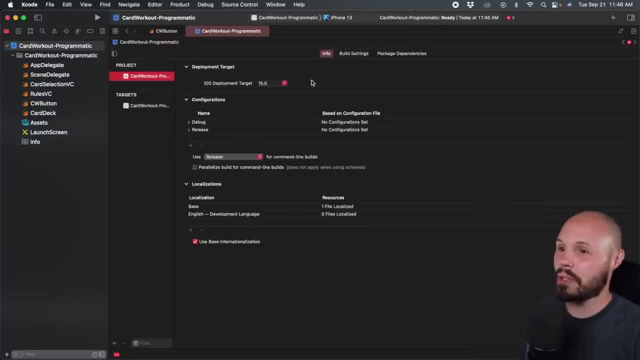 to make sure you don't run into that issue, Anyway. so now that we're supporting iOS 15, back to CW button, Let's do a command B to hopefully get rid of those errors. Okay, well, we got plenty of other errors. 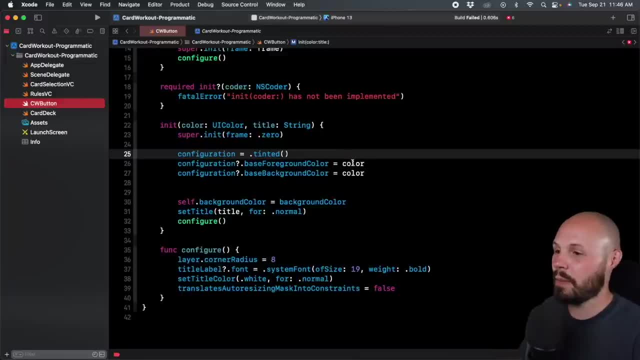 because we're in the middle of revamping our buttons, but we took care of that one, So we have the background color and the foreground color. Now let's take care of some of the other properties. right, We had the corner style property, right? 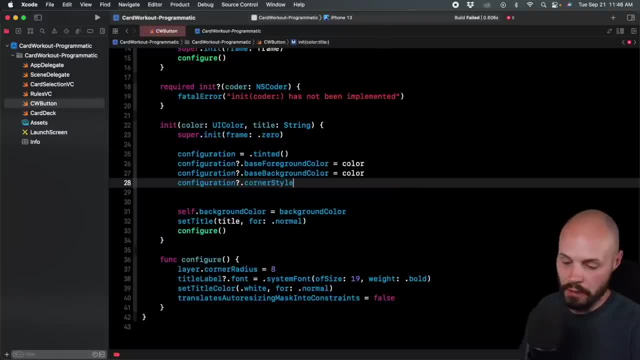 Our corner radius, So configurationcornerstyle equals. and then, if I do dot, remember, medium capsule, dynamic, small, large, do whatever you like, but we're gonna go with medium. And then that sets the base status of the button. 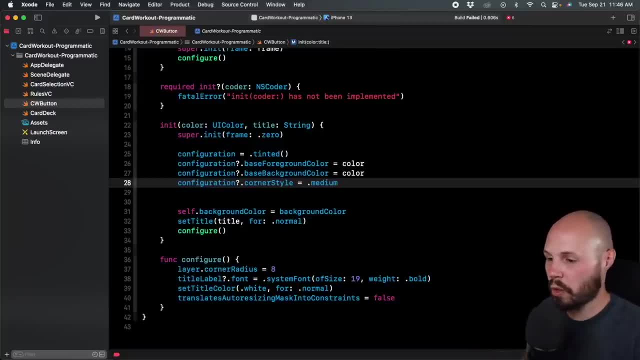 So actually, let's pause here before we do the image and make sure that we get to the bottom. So let's pause here before we do the image and make sure that we get to the bottom And make sure this is all working. get this going. 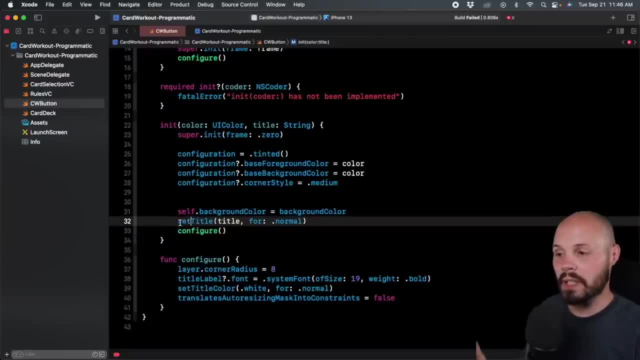 So before we add the image, I can get rid of all the not quite look set title. That's what we're not doing yet. See, we're passing in a title but we're not setting it, So I can do that here. 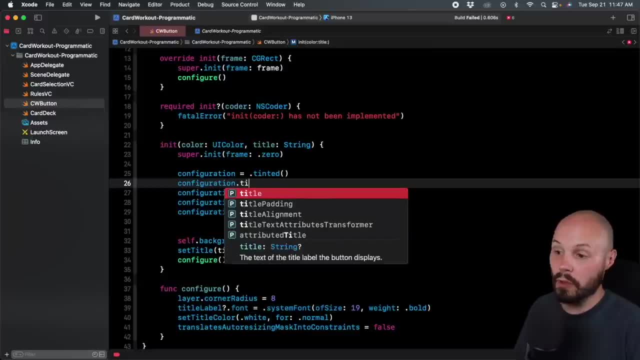 I'm gonna do that at the top, cause that's pretty important. Configurationtitle: there you go, equals title, And that is whatever string we pass in. we're setting that title. So this is actually a good way to check as well, right? 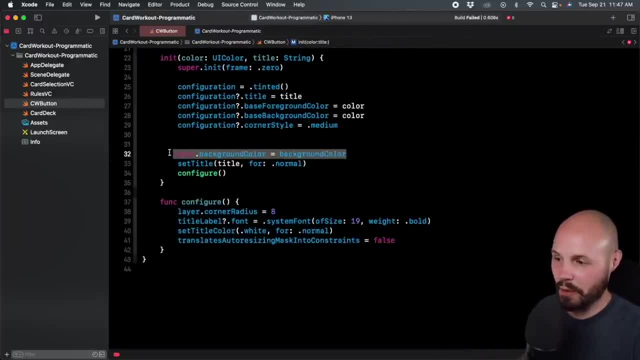 Before you delete the old code, make sure you're handling it. Well, we're handling the background color, cool. We're handling the title and then configure, which is down here. We need to make sure we handle all of that. Okay, so let's delete that. 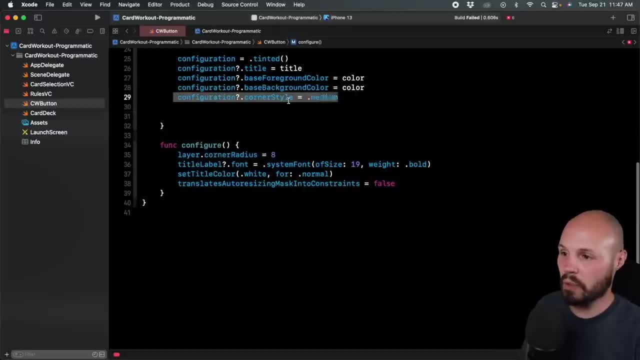 Let's take a look through the configure method. We're handling the corner radius right In our corner style. cool, Can delete that, Can delete the font. that is the default. Again, we're working with like default Apple style right. 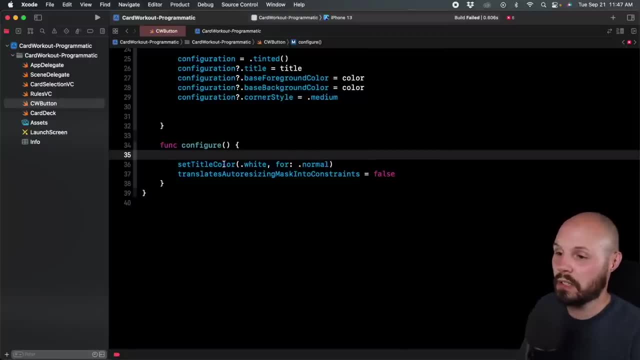 That's the trade-off you make when you go with these configurations. Set title color: that's our foreground color. setting our font color Translates auto or Tamek, whatever. We're still gonna need that, So I'm gonna bring that up into our initializer. 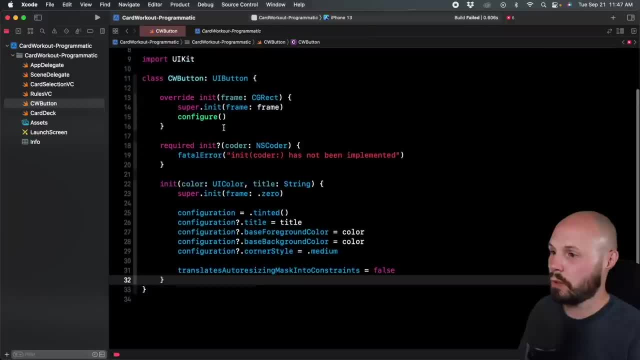 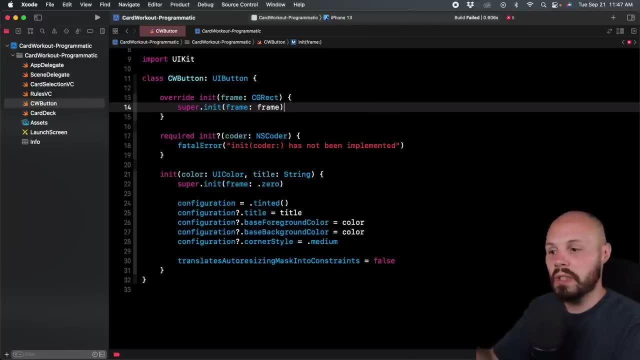 and then I can delete this configure method altogether, which will remove it from up here as well. So we're simplifying our code because, again, the trade-off is we don't have to set all this stuff ourselves. We're using these configurations to get the default Apple look of the tinted style. 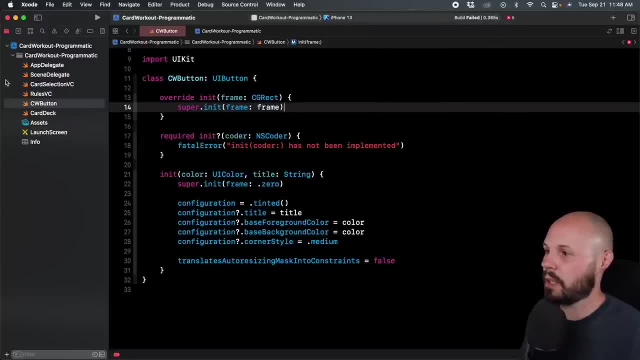 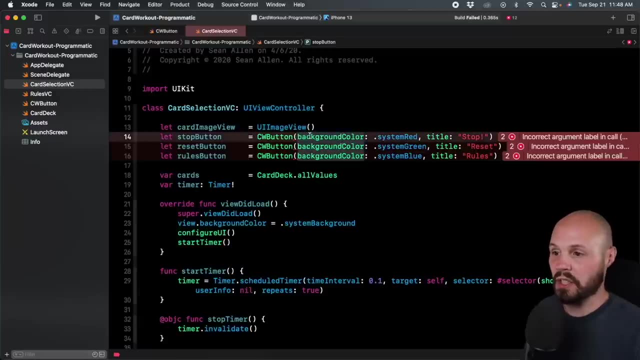 So we'll do a command B and we have six errors. So that's gonna be in our card selection VC. And you see, here is because we changed the initializer of our CW button right, It's not background color anymore, it's just color. 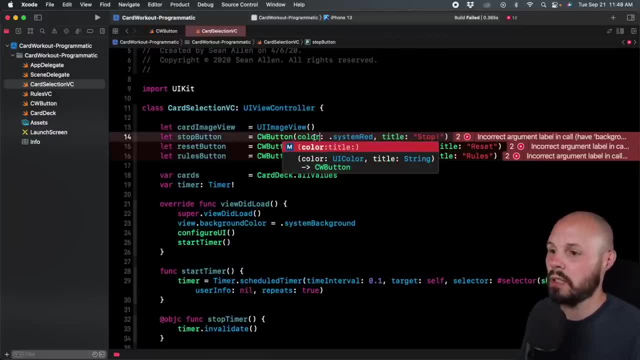 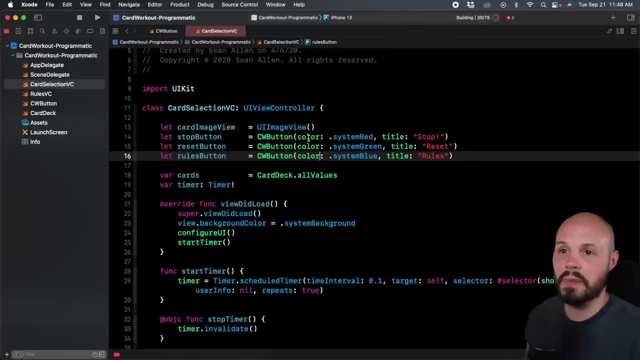 So what I can do is change this to color. double click to copy. double click, paste, paste. Do a command B. All we do is just change that to color. Okay, that should work for now, And once we make sure we have no errors, cool. 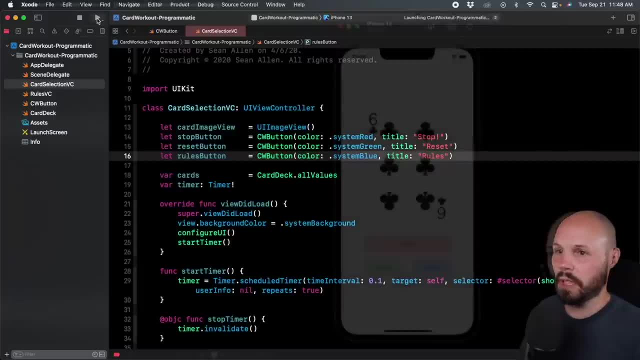 Again, this is just checking to make sure it works before we add our images. So I'm gonna run it And here you go, our app is running. We haven't set our images yet, but you can see our buttons are now that default tint style. 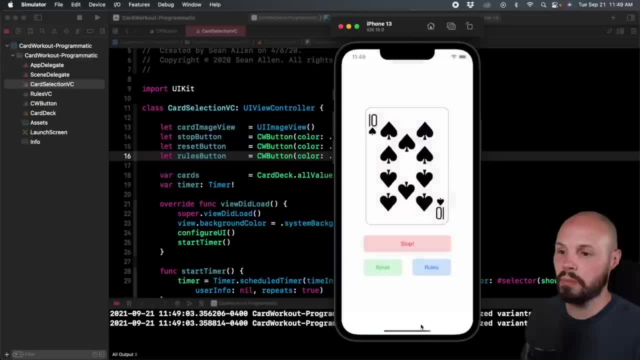 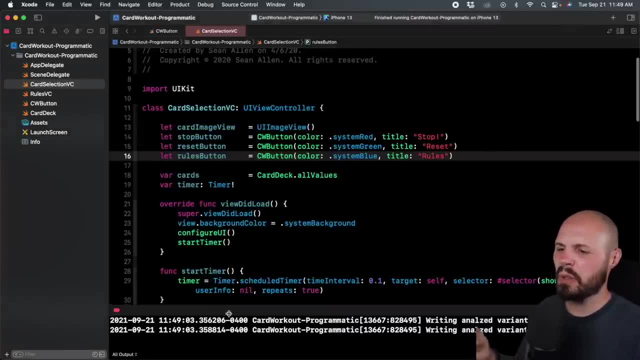 and they still work. right, Stop, reset rules, cool, Okay. so everything's still working. Now we just wanna add those images, like we did in the storyboard version, right, Okay? so stop there. And it is always good practice to kind of like: 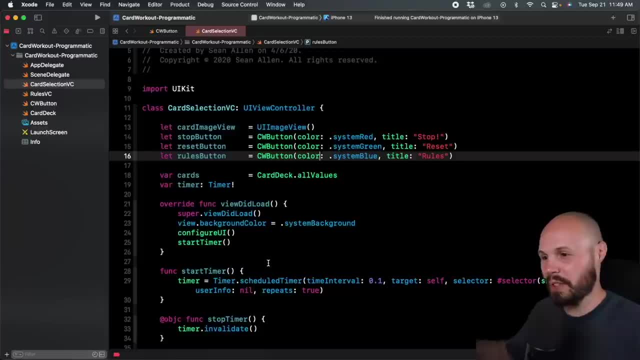 check to make sure your stuff is still working along the way, rather than building forever. That way, if there's a bug like, you know where the bug is if you kind of run it to make sure things are working. So we know we got our button working. 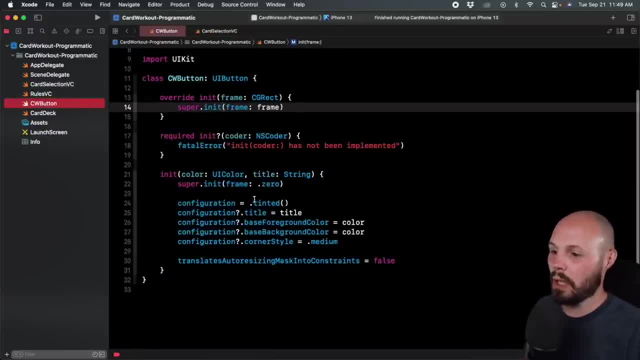 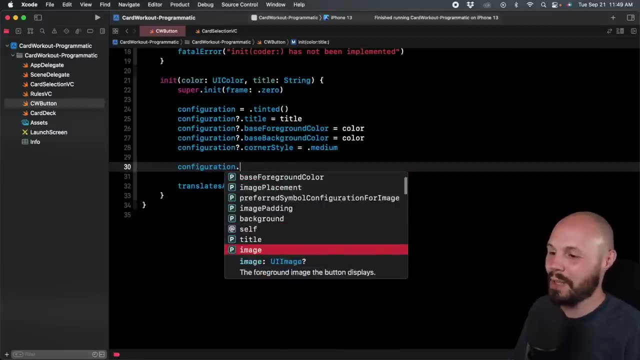 with just color and title. Now let's add the image back to CW button. Again, it's just more configuration stuff, right? So configuration- I don't know why I put it on a separate line, but we can do image right. 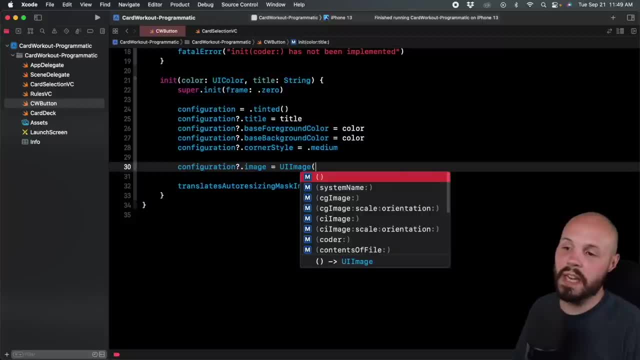 And that is gonna equal a UI image And then the initializer on that is: this is new. I don't think we covered this before. system name- right, You're gonna see one just called named. I think we did that before. 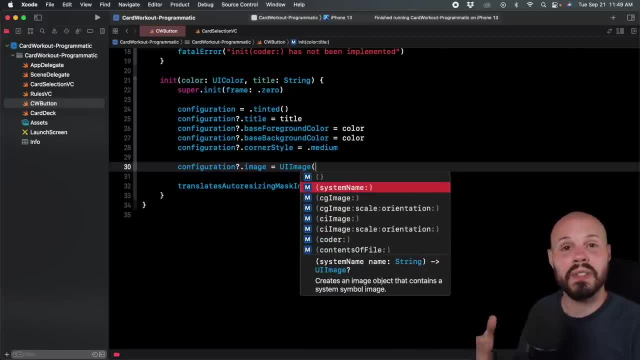 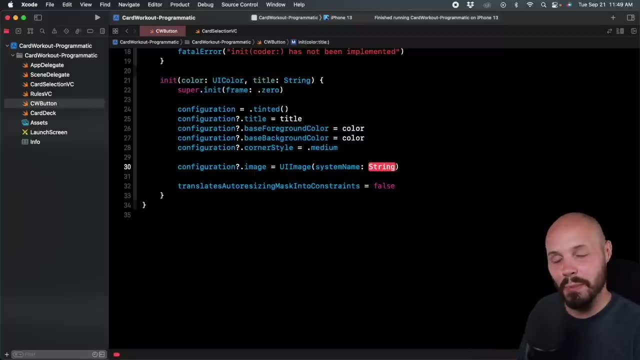 We want system name, And what system name is that gives us the SF symbol that I mentioned before. Now in the storyboard we just had the dropdown and we got all that kind of for free. SF symbols was kind of built into storyboard But for us to look at it it's a separate program. 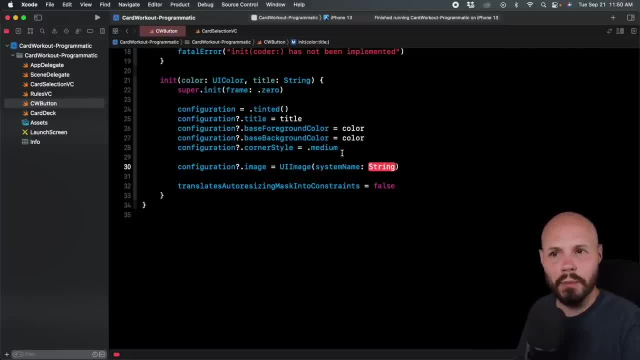 You can just copy the string that I do. I'm gonna link to my video, YouTube video on SF symbols That does a deep dive. I don't wanna derail this path, cause all you really need is the string, But to find the string we need to go into SF symbols. 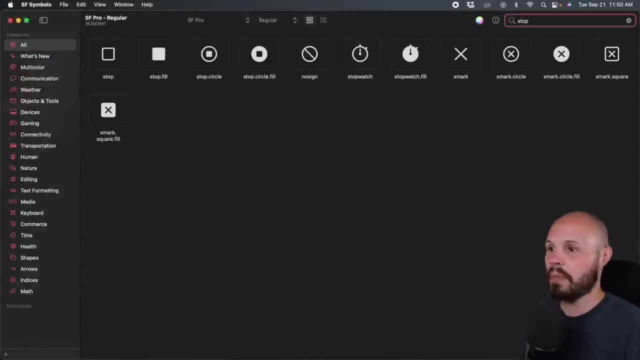 So here I am in SF symbols. right, Just like we did on storyboard, I'm gonna search stop. Here we go. I got the stop in a circle here, So you see it's stop dot circle. You can do command shift C to copy. 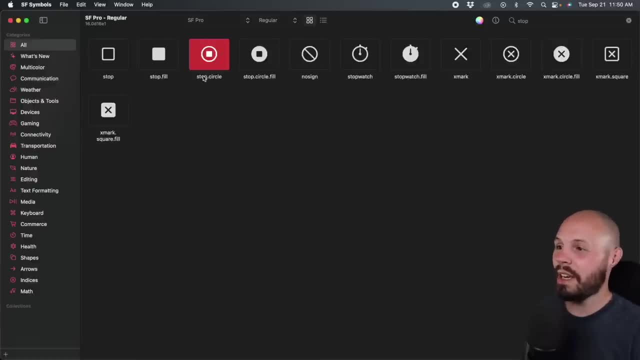 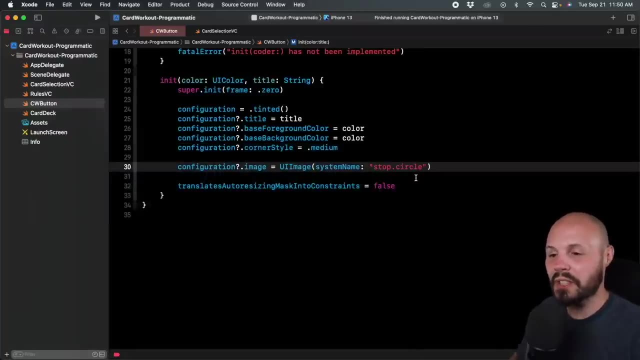 Command shift C, not just command C, Command shift C to copy, And that'll give you stop dot circle, Or you can just remember stop dot circle. I like to copy and paste, just in case. So there you go, Or actually you know what. 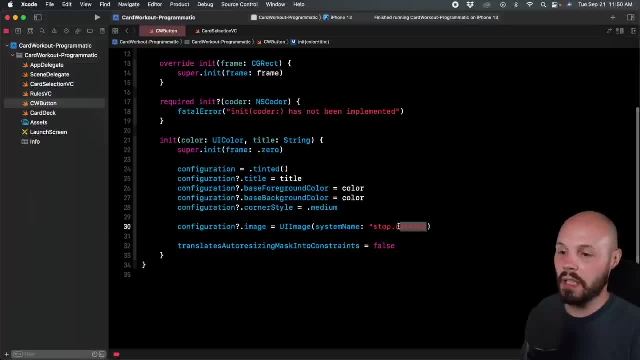 I'm silly. We don't need to put that in here now. We just need to pass in an image name, right, Because these buttons are dynamic, right? Whatever image name we pass in, that's what we're gonna set. That would set all of my buttons. 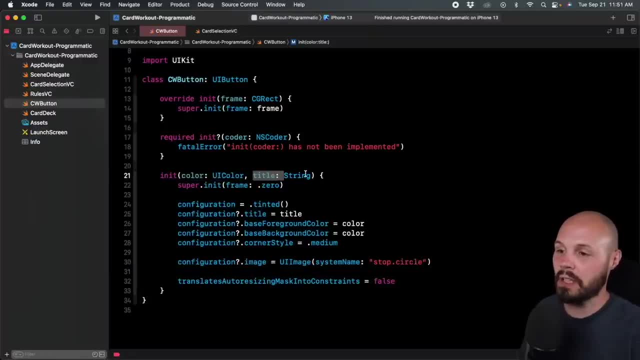 in a circle. So I need another parameter here. I need to pass in color title and then I'm gonna call it system image name. That way I know it's an SF symbol and I don't just pass in a random string. 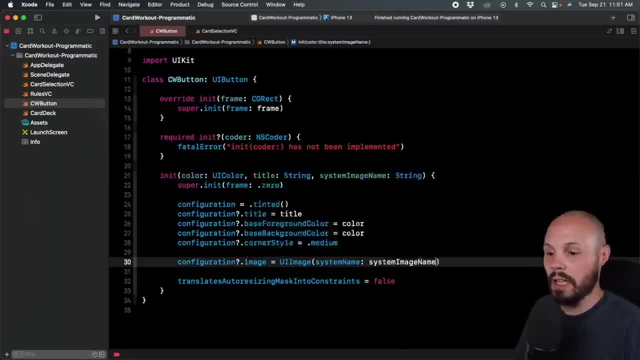 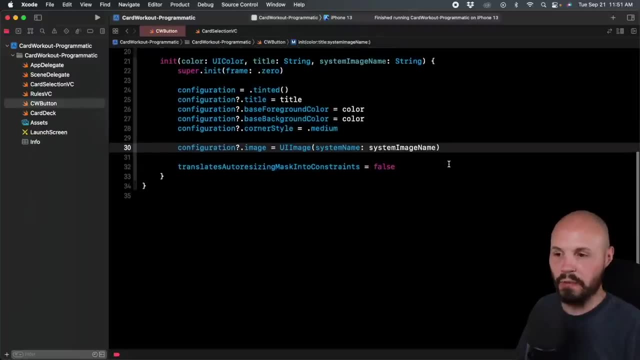 So now, instead of stop circle here, I'll do system image name. So that way, whatever image name we pass in, that's what the button will populate, And then I'll scroll up a little bit And then just like before, right. 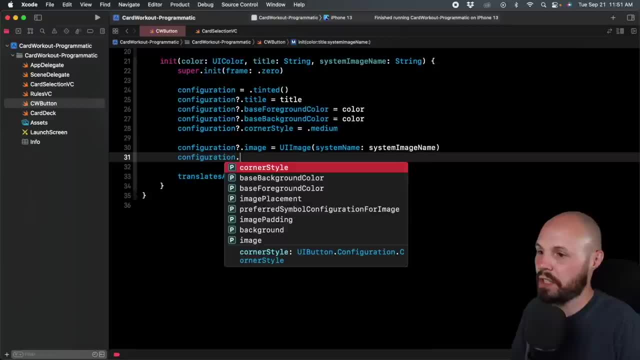 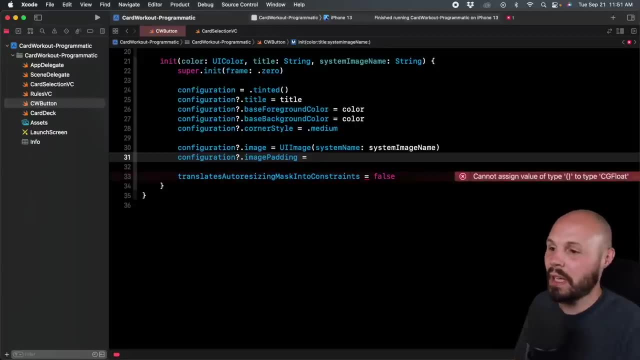 We needed to give our image some padding right, So we did configuration dot image padding. There you go, And this is all doing the same stuff that we did in storyboard, Just do it in code. So now we'll just give it a five. 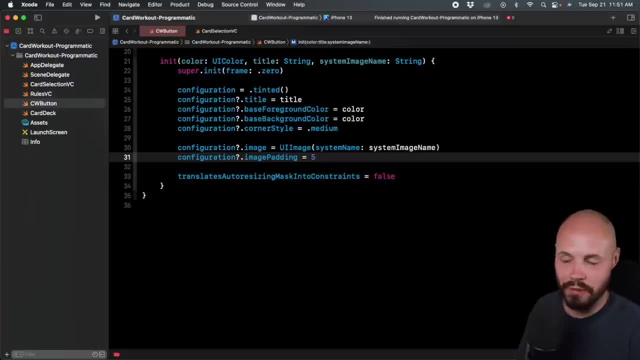 And you can tweak this number to get the padding you like. Remember how we were just tapping the arrows in storyboard? Or you're just entering a number here. And then, lastly, something we didn't cover in the storyboard but I'll show you here. 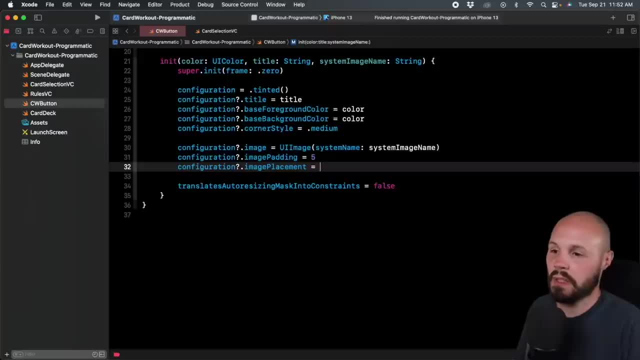 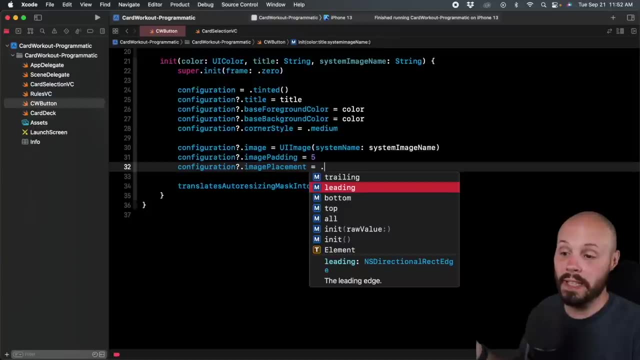 We can do image placement right. And what is image placement Dot? you can see I can do trailing leading, bottom, top. So before our image was to the left of the title, right, That would be leading And I think that's the default. 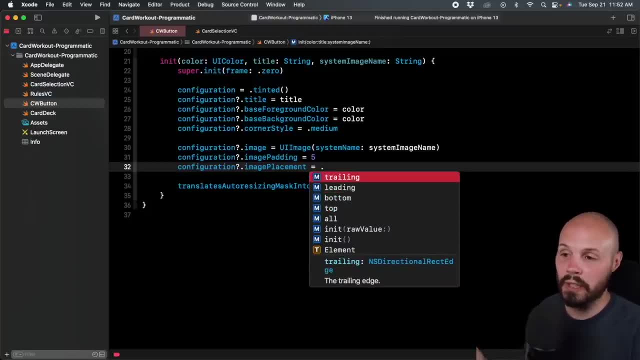 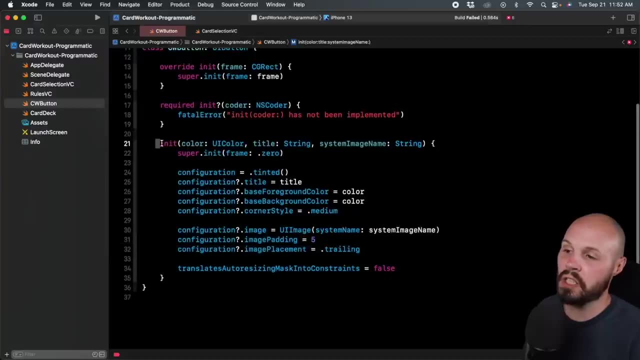 Well, you can make it. you can put the image on top, You can put the image on the bottom. trailing, We'll do trailing, just to show you what it is. And now you should see, we're gonna get some errors because we changed the initializer on our CW buttons, right? 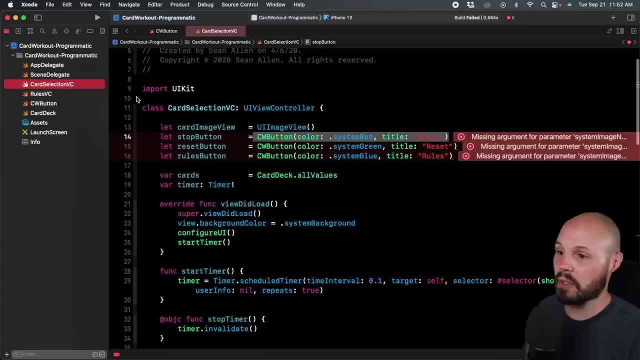 We're now passing in a system image name. So if I go to my card selection VC, yep, it's saying we're missing the argument: system image name. So let's add that here, fix, Okay. so the red stop one again was: 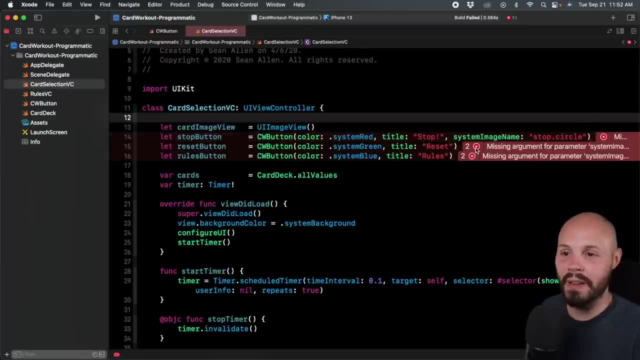 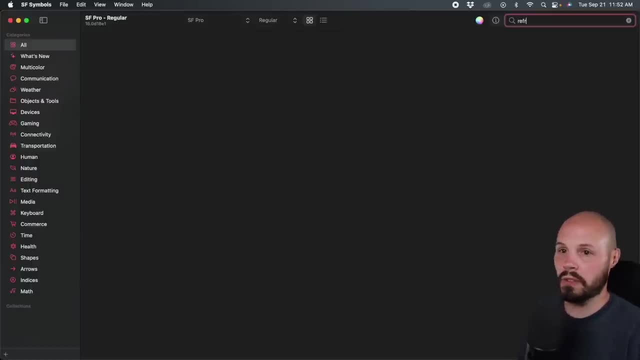 we'll paste this in now: stop dot circle right, Remember we looked that up. So reset. Let's go back to SF symbols And I will search for refresh, just like we did on the storyboard. No, oh, there it goes. 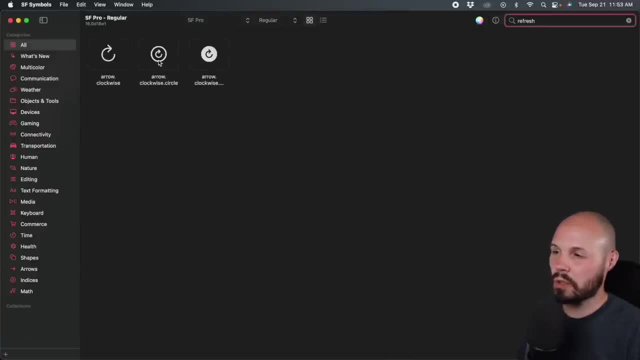 Took a second And that was the arrow clockwise circle. I don't think we did the circle last time, but we'll stay consistent. So command shift C. Now you can see why I wanna copy these, cause that's quite a long name. 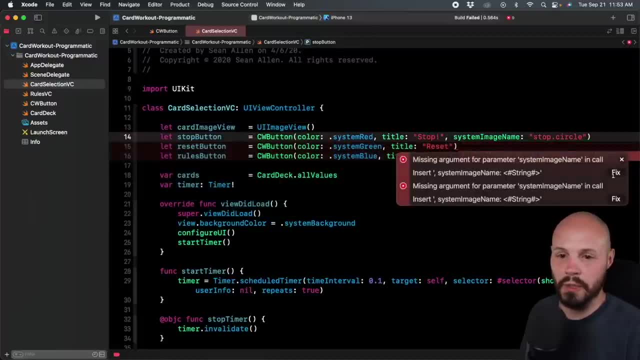 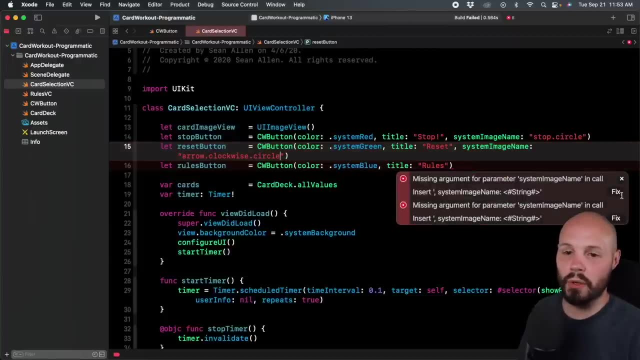 Alt tab back to Xcode, And then we'll add the parameter here, fix, And then the string we wanna do is command V for arrow dot, clockwise dot, circle, And then we'll do the same thing for rules, which we had a list. 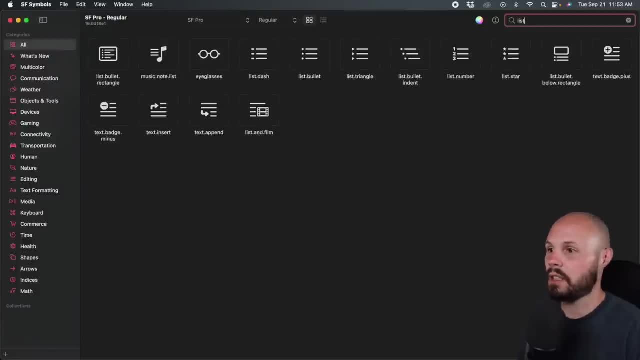 Not sure. if there's a circle version of list, We'll see here List. no, there is no, that wasn't. we got different lists before. Who cares, I won't waste the time with this, but we'll do list dot bullet. 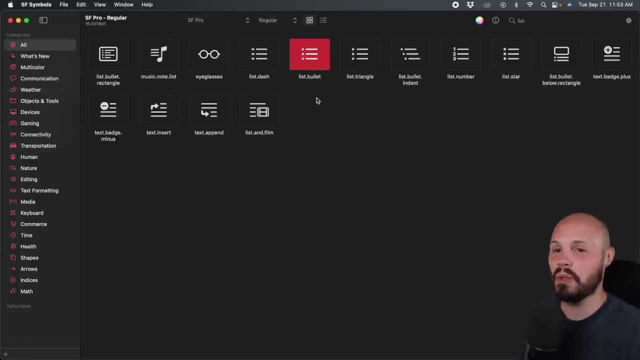 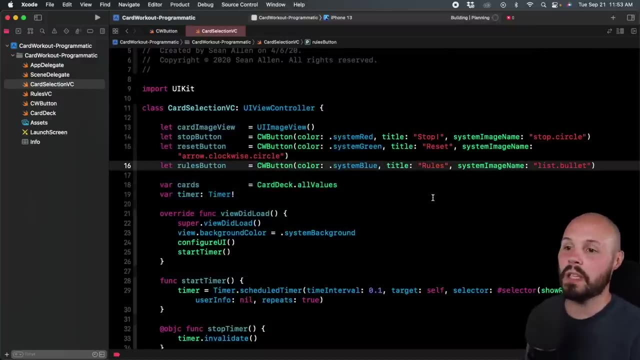 And again we lost our circle consistency. but you can play around in SF symbols and find some symbols you like to style your buttons here. Command V, list dot bullet. do a command V. Okay, so now again our initializer on our CW button. 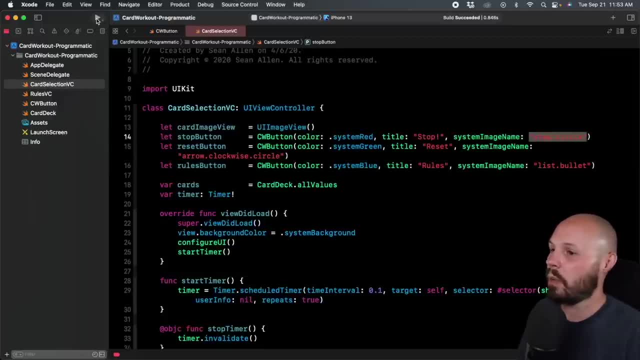 now takes in a system image name which we passed in, And now when I run it, we're gonna see the images on the trailing side, right Cause. see how we set it up. Now they're to the right. You could put them on the top. 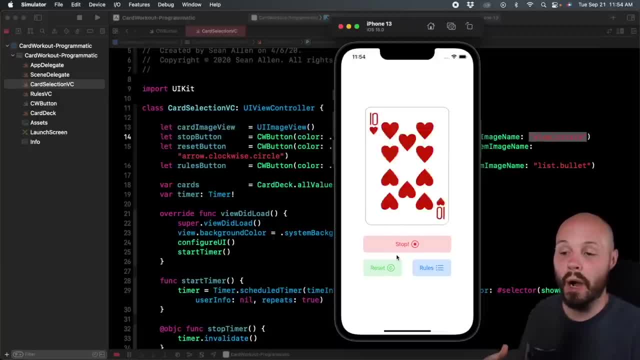 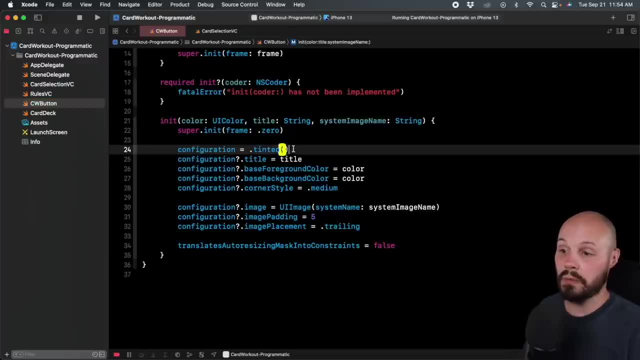 You could put them on the bottom, You could put them on the left. So that's more customization on these buttons. So again, that's the new button configuration in code. Quick review: here Again, we just created a configuration. We did dot tinted. 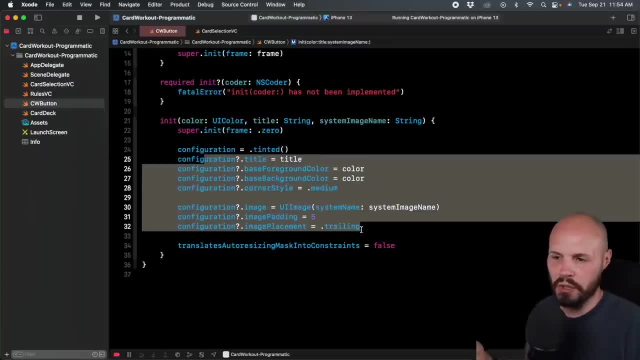 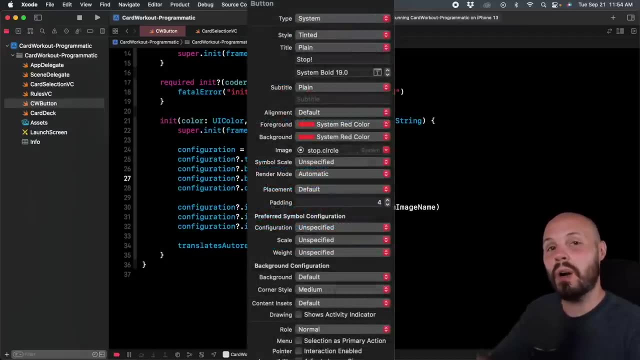 Again, you could do dot filled, dot gray. You would have to change your styling based on that. But based on our tinted styling, we set title foreground color, back color, all those properties you saw on the right in the store. 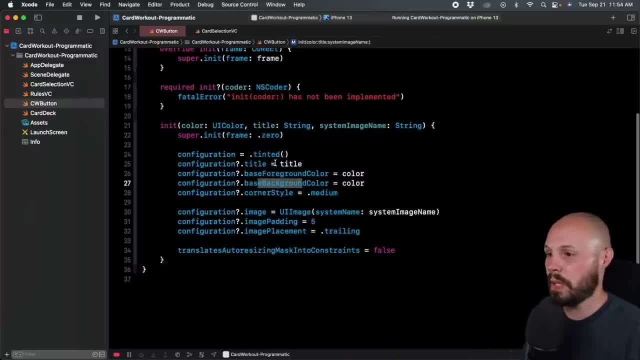 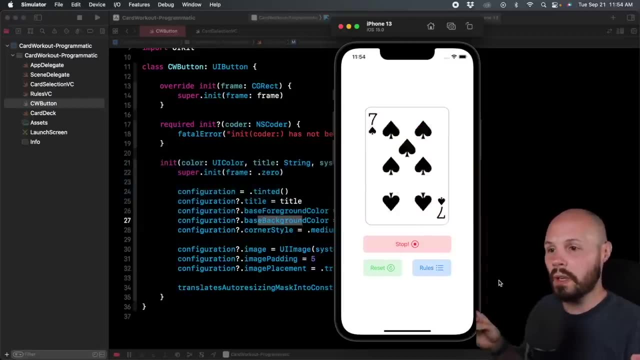 storyboard are here in code as well, So you could do it this way, whichever you prefer. And then, as you saw, our app is running as expected with the new styles, So hope you enjoy the new buttons in iOS 15.. I think it's a great way to get that default Apple look. 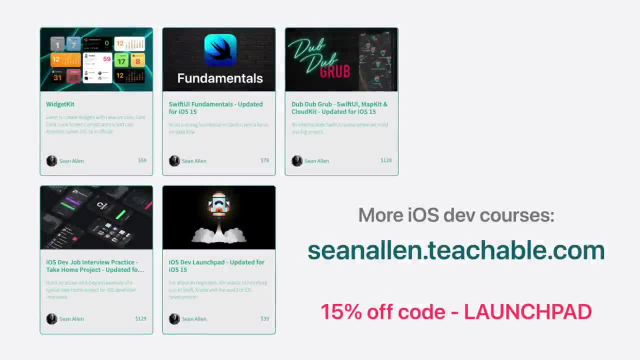 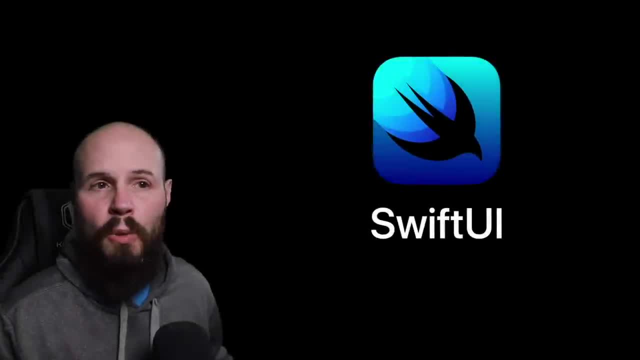 and we don't have to build it ourselves anymore. Over the next two videos, we're going to be previewing SwiftUI, And I wanna stress preview, because this is not meant to be a full blown tutorial on SwiftUI Like that. is an entirely different course. 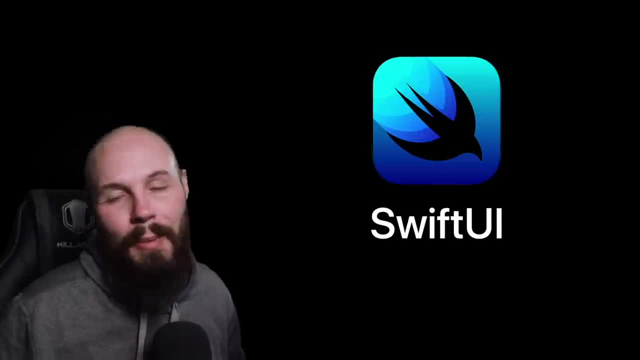 not just one or two videos. So I wanna set those expectations and I'm gonna say it again in the next video. But anyway, like what is SwiftUI? So, as I mentioned in previous videos, SwiftUI was introduced to us just in the summer of 2019. 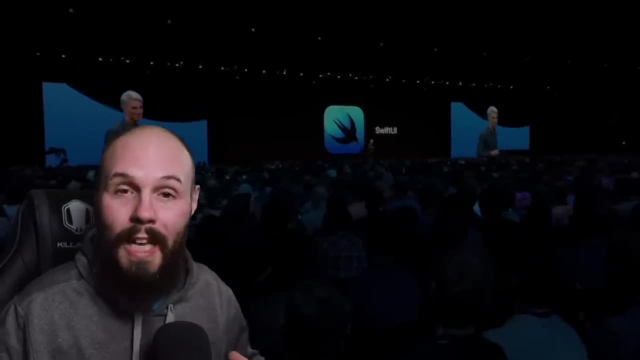 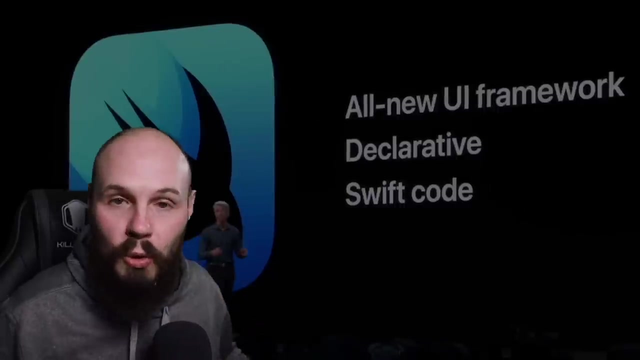 at WWDC. So that's when it was announced. By the time it was like officially released and out of beta, it was late September of 2019.. So here it is, Here in early April 2020, it's only been released for six months. 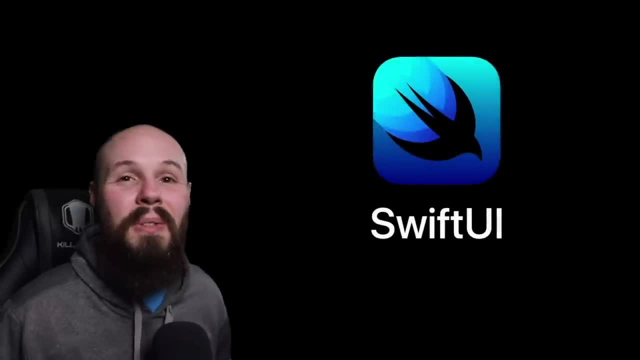 So it is very, very early in the game And this is a fundamentally different way for us to build our UIs, not only on iOS, but across all the Apple platforms right: MacOS, iPadOS, iOS, watchOS. And I wanna go back to how early we are in SwiftUI. 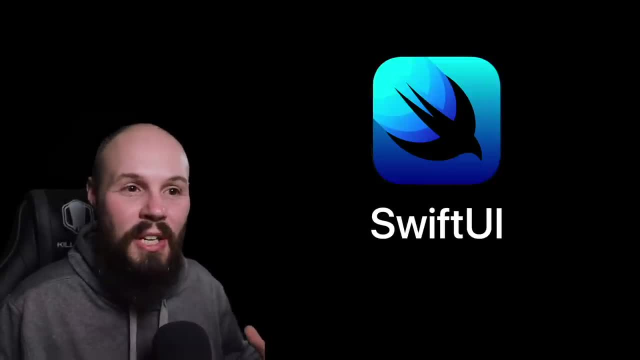 just to stress that, because I know, especially after watching these two videos, you may get really excited about this and want to only learn SwiftUI. But just to reiterate what I said in the UI kit or SwiftUI: we're in a transitionary period. 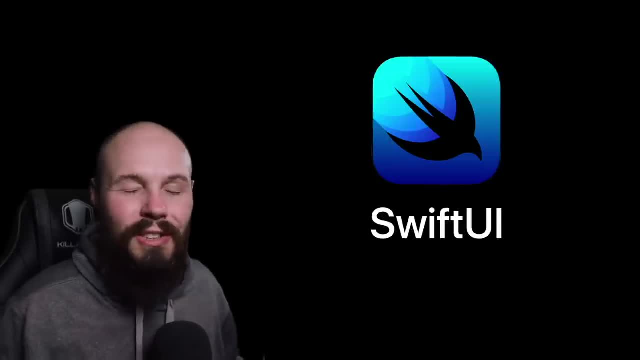 that if you're trying to be an iOS developer in the next two, three years, you're gonna have to know both again because we are in that transition period. But before we go any further, I would recommend, especially since this course is for absolute beginners- 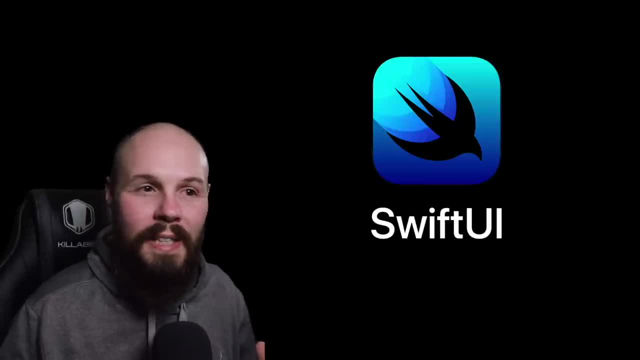 learn one at a time, Like it's fine to know what SwiftUI is and to like maybe play a little bit, but I don't recommend splitting your time 50-50.. I would learn one and then learn the other And I would learn UI kit first. 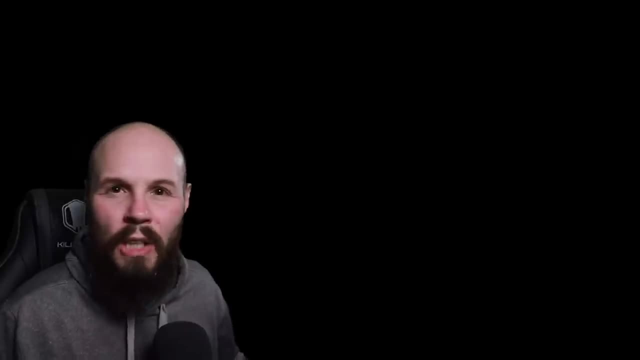 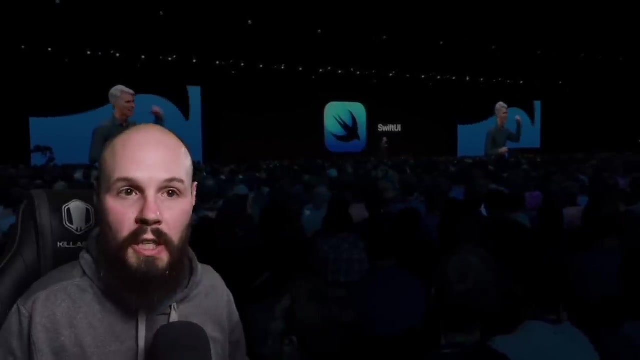 because all those best practices and how we do things in UI kit are well established. The thing with SwiftUI: because it's so early, like for the past year. so here in June of 2020, it will be the one year anniversary. 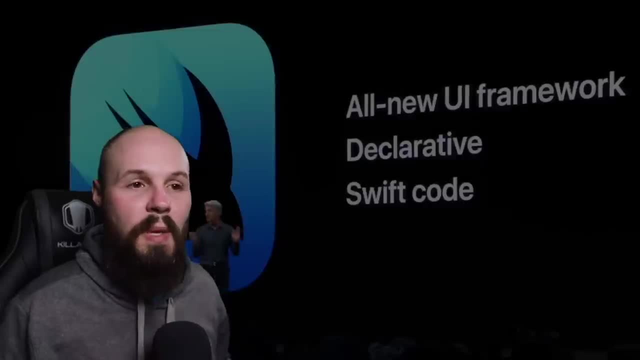 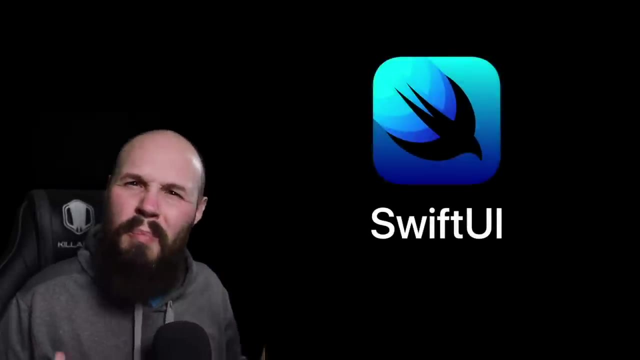 of when SwiftUI was announced. So developers in the community have spent the past year like trying to figure it out. Like we as a community don't know all the best practices yet Don't know what's the best way to build a SwiftUI app. 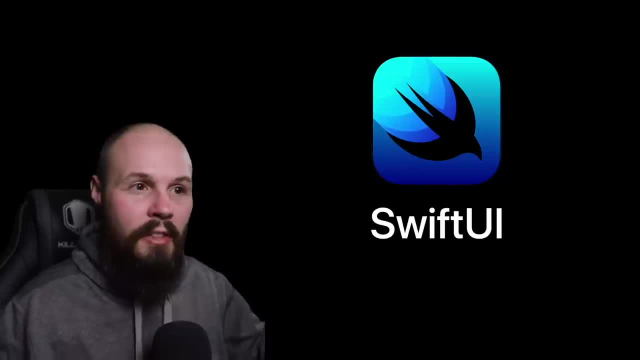 And because, we don't know, there's a lot of experimentation going on. The SwiftUI space is going to change drastically over the next couple of years. So that's why I recommend learning UI kit first, because if you start trying to learn SwiftUI now, 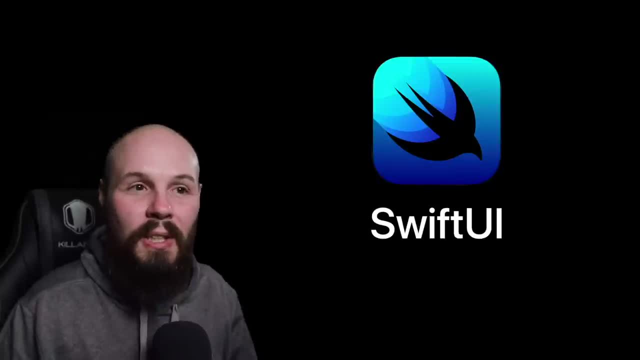 it's going to change and evolve so much that for a new beginner like that's a lot to keep up with. All right, now let's move on to like what it is and start talking about the overview. So here I have, up a website from Apple. 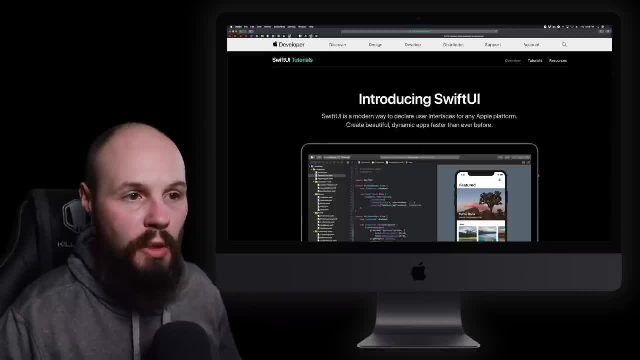 I'll link to it in the description, of course, But you can see here introducing SwiftUI And, before we go any further, I'm sure you're going to be very interested in this. You can see this says SwiftUI tutorials in the upper left. 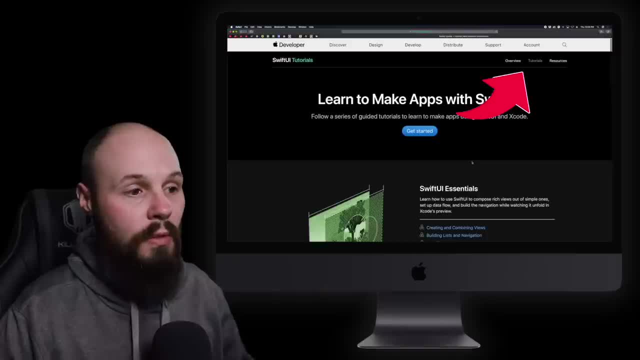 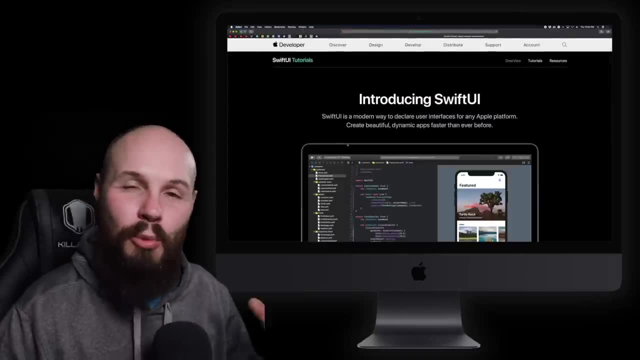 And if you click on the right here tutorials, you'll see a whole list of SwiftUI tutorials that Apple has created just for SwiftUI And they're very, very well done. The community was super impressed by the SwiftUI tutorials Apple put out. 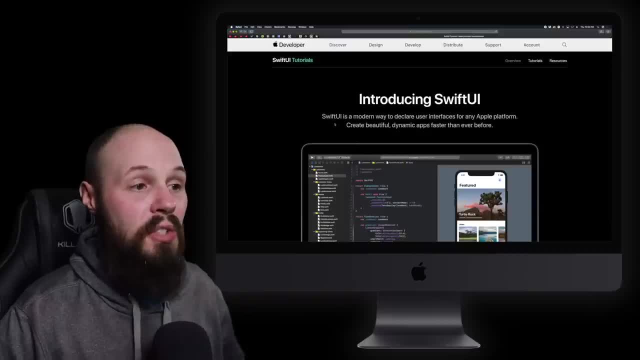 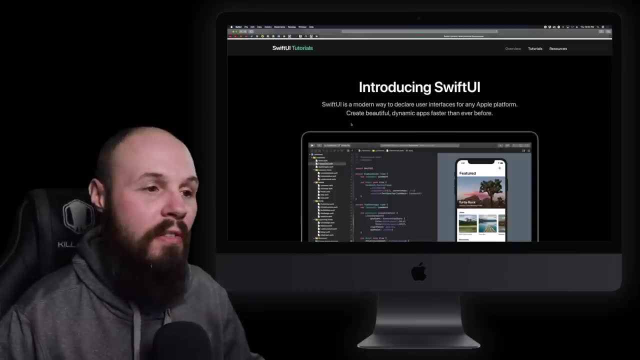 Let's just say it is far and above what they usually do. So here you can see. SwiftUI is a modern way to declare user interfaces for any Apple platform. Create beautiful, dynamic apps faster than ever before. The key word I want to hang on here is: declare right. 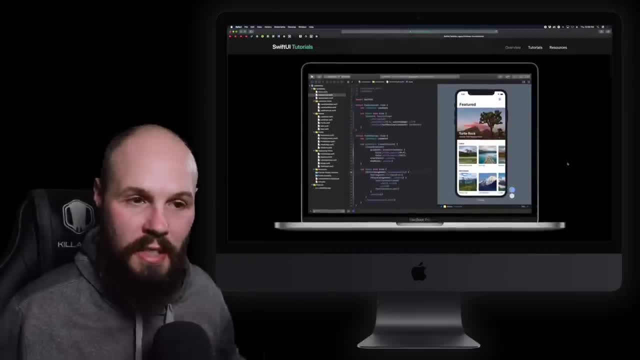 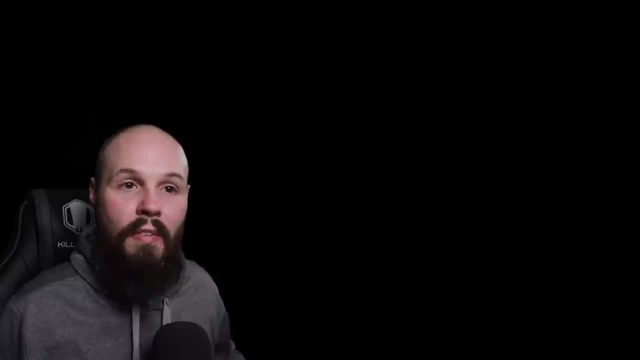 So let me put up this picture here so you can kind of see what's going on as I describe this. So the major fundamental difference I was talking about is in programming paradigms, right, So you have imperative programming in declarative programming. 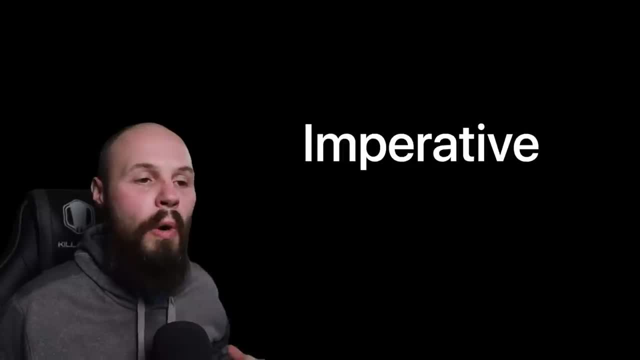 The way UIKit works is imperative At a high level. the way imperative programming works is you tell the computer how to do something right. Think back to our card workout app, like even just the ViewDidLoad in our list of functions. We're telling the app or the computer. 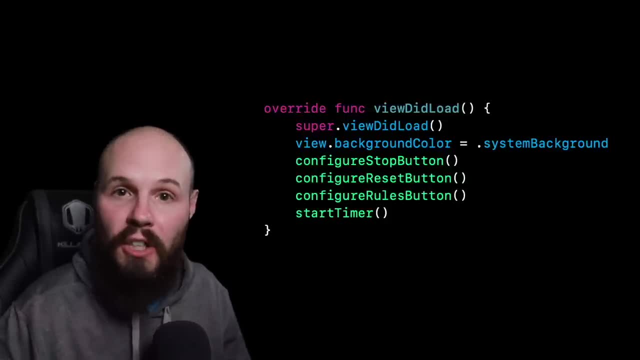 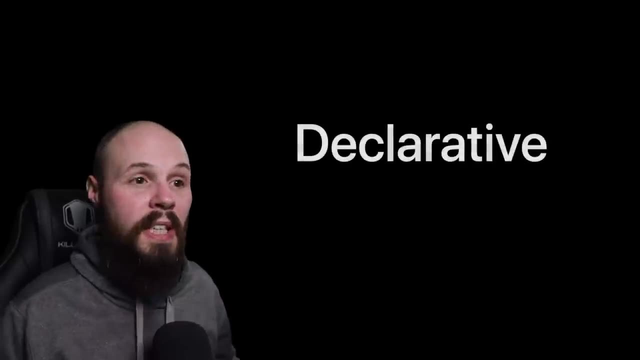 exactly what to do and how to do it. That's why we're declaring all these functions and we're saying, right, run this function, then run this function, then run this function. right, we're telling it how to do things, whereas declarative is where you kind of define or declare what you want to happen. 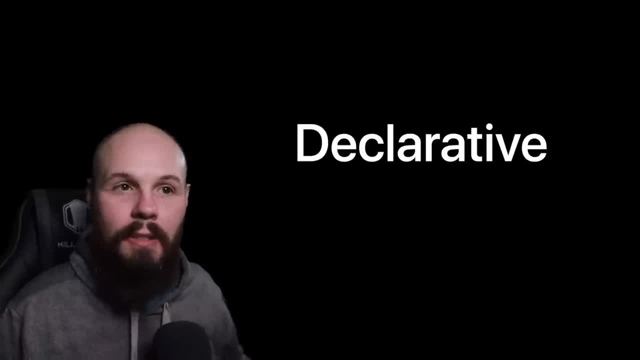 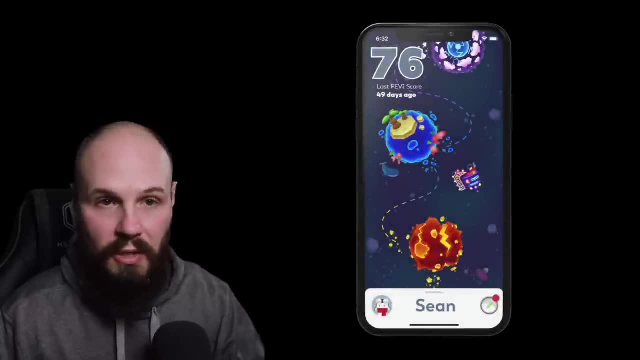 and then the computer like figures out how to make that happen. let me give you an example. so say you have two screen states, right. one is: if the user is logged in, you're going to show this ui on the screen, the home screen. if the user is not logged in, you're going to show the login screen as you. 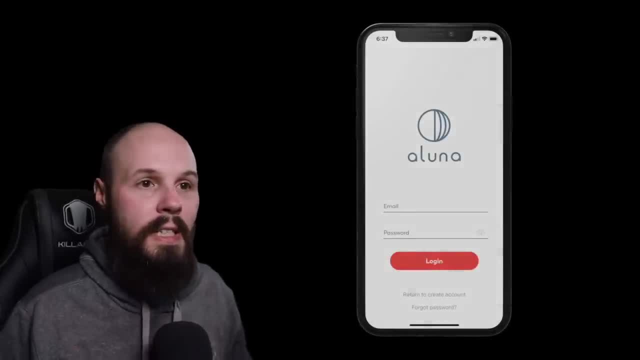 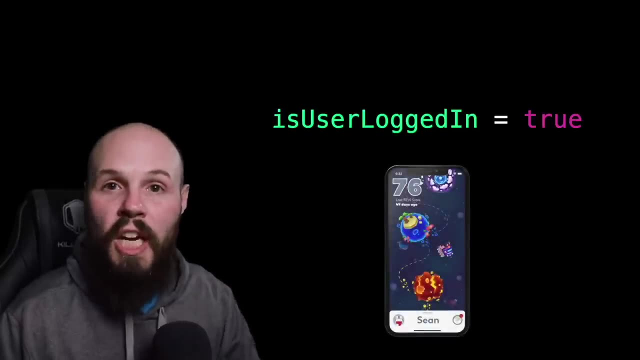 see here. so all you have to do with declarative ui is change the state of the screen, which is typically like an is logged in variable to on or off and based on that variable changing. that is how the ui knows to update. it's kind of like watching that variable: that state is logged in. 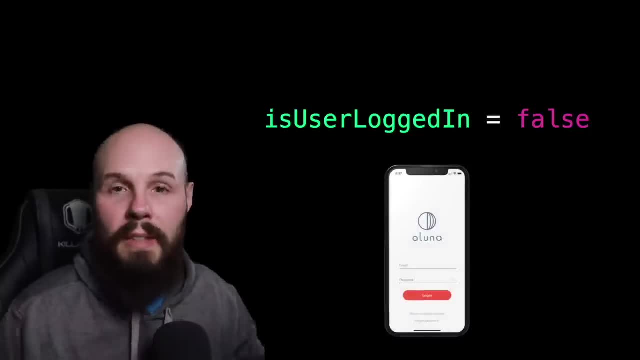 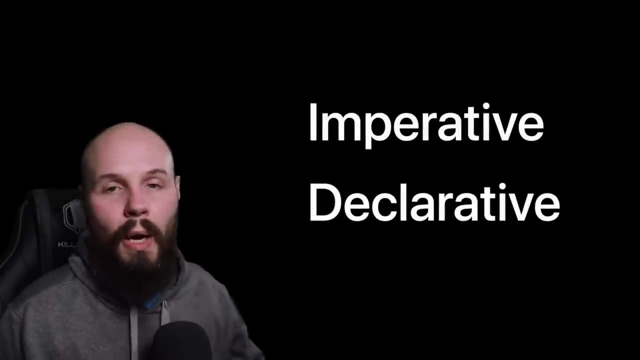 and then, whenever you change it, it reacts to that change and automatically adapts its ui. so again, that's super high level imperative versus declarative. but that is the fundamental difference between ui kit and swift ui, and i want to stress how, how different this paradigm is, because even experienced developers that haven't dealt with 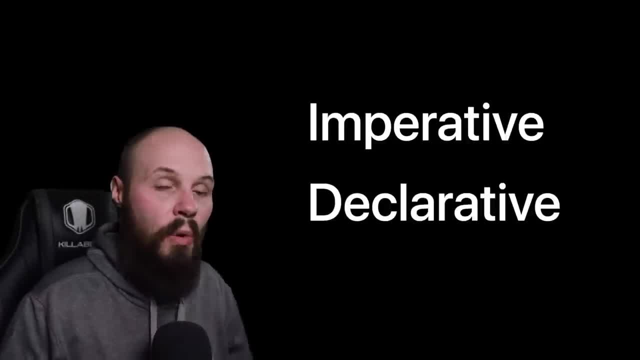 reactive programming in the past or declarative programming. languages- um, we're all beginners like this is brand new and you know i've done my fair share of courses and playing with swift ui and learning and it was just like being a beginner again. like i use this analogy right, it's like 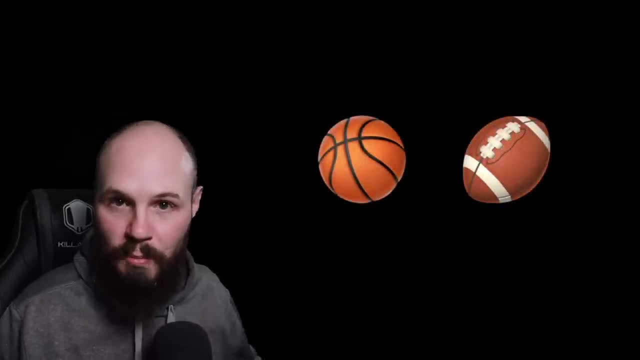 sports. um basketball and football. yes, they are both sports. so being athletic, a fast runner, like sure, that skill carries over. but once you get down below, you know basketball and football are completely different, completely different skill sets. so that's the analogy, right, like sure, declarative and imperative. or ui kit and swift, ui, you're still programming. so 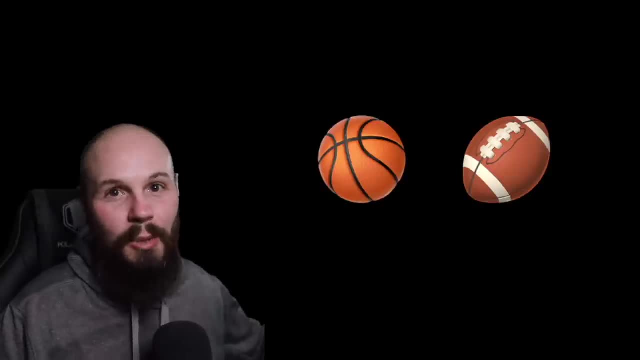 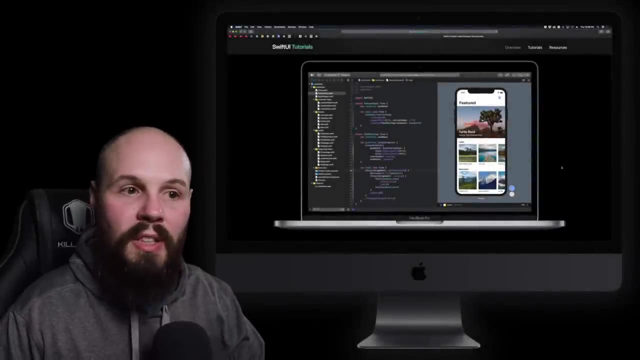 general programming skills help, but it's like playing basketball versus playing football. right, they're totally different. so, all right, let's keep running down this website, but what you're looking at here is you have the code on the left and the canvas on the right. um, so this isn't storyboard. 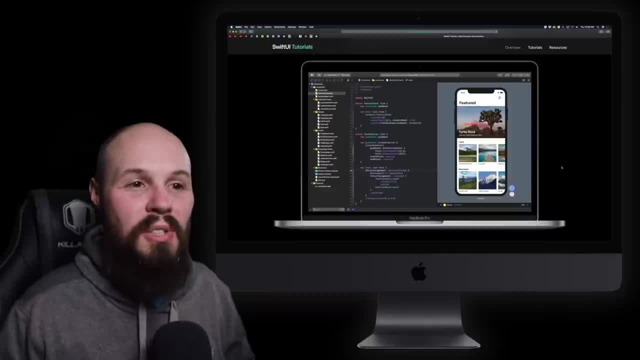 even though it kind of looks like storyboard. um, the way this works is you? you kind of get the best of both worlds. you'll see, in the next video i'm going to show you how to do that. so let's get into the next video, when we actually build a sample app that, uh, you can either do stuff on the canvas. 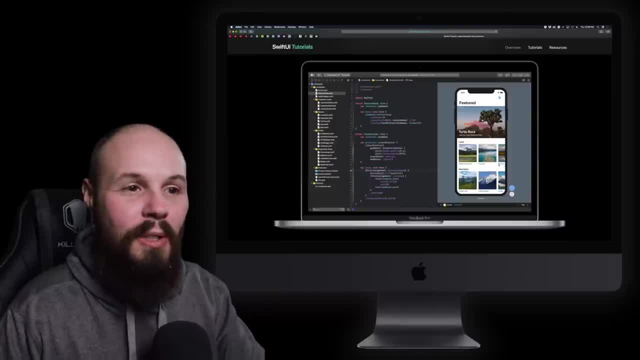 so it kind of feels like storyboard. and then what happens? when you drop something on the canvas, it automatically populates the code over in the code. so if you're the type that just prefers you know type, not the code, no canvas, cool, you can do that. if you're the type that likes to be visual. 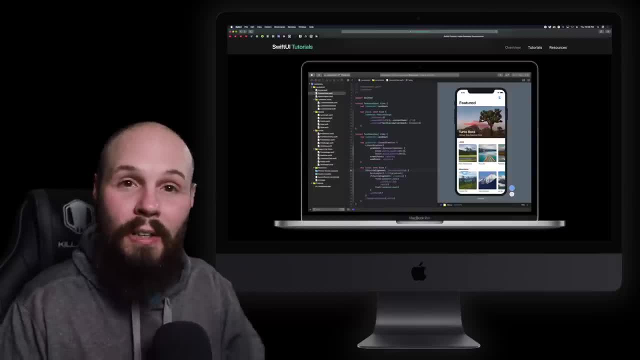 and drag and drop on the canvas, that will work too, and then when you drag it on the canvas, it'll spit out the code. it's actually kind of crazy, and again you'll see that in the next video. so the canvas here is an amazing part of swift ui. it's not just a little bit of a trick. you can do it in a couple of ways. 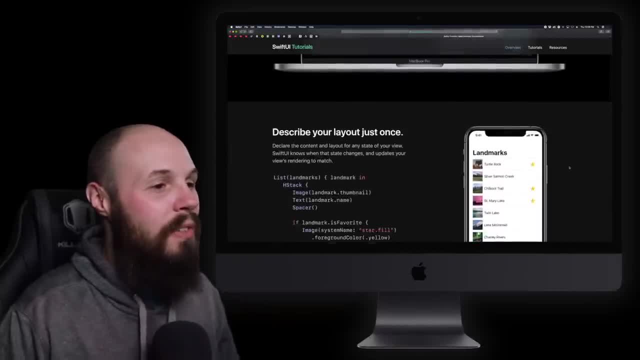 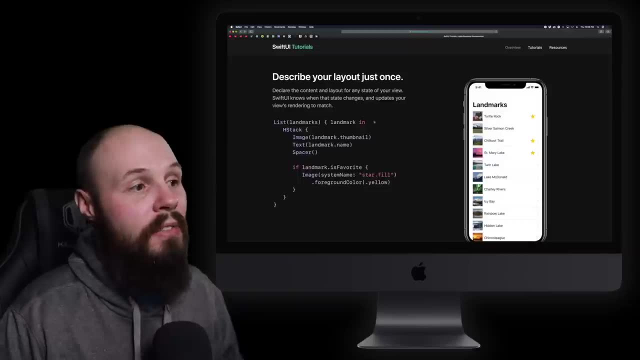 part of swift ui again. you'll see it in action in a bit. let's keep it moving. so describe your layout just once. this is what we're talking about with declarative. that says: declare the content and layout for any state of your view. swift ui knows when that state changes and updates your views. 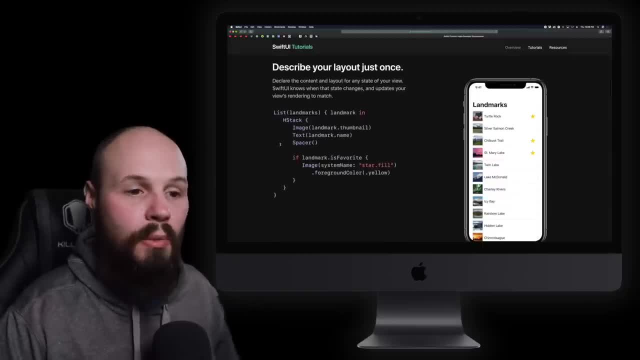 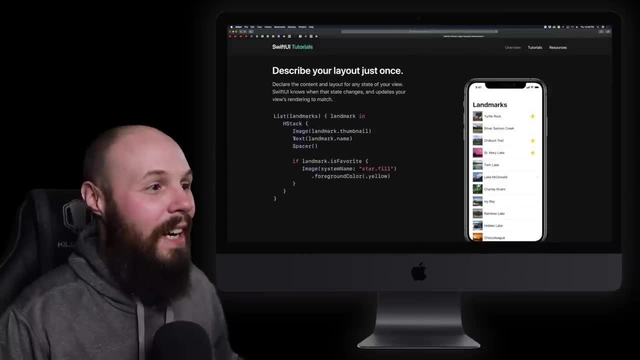 rendering to match. and just as an example, like: see this table view on the right: i'm scrolling up. it won't scroll up any higher. i know the non-vertical centering bothers me too, but it won't do it. see, i'm moving this, it's not moving. uh, anyway, this code right here. 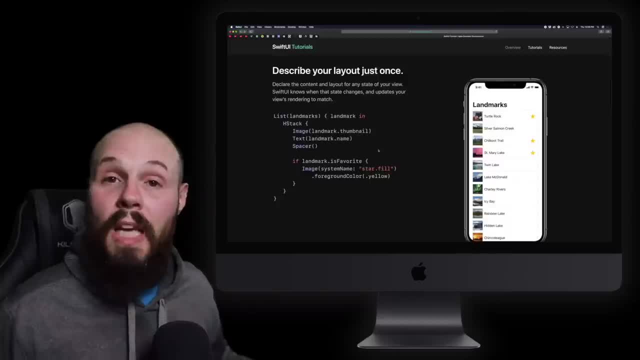 this is all the code it took to populate this table view. now we've built a table view in our colors app. remember all that you know. we had to set the delegates, we had to put the table view on the screen, we had to set the constraints to declare it. none of that right. 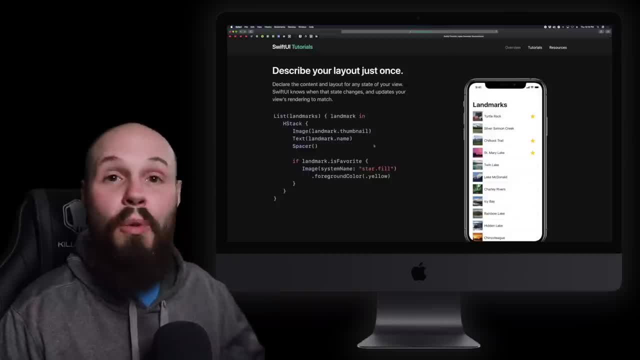 there's no constraints in swift ui, and let's walk through this code real quick to give you an idea now. don't worry if you don't get it. we're actually going to dive into the code in the next video, but i'll walk you through this. so this list is basically our table view. right a list. look at the. 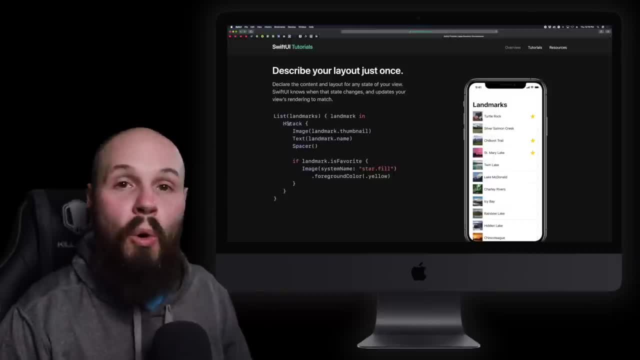 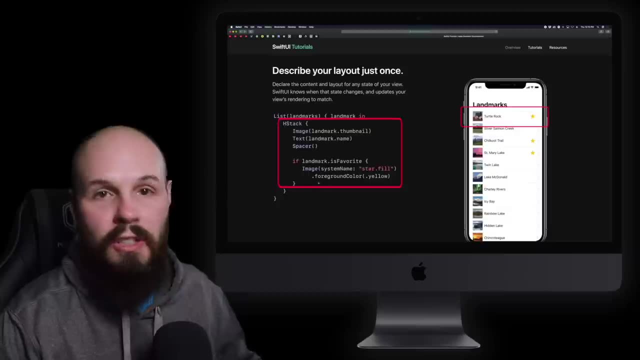 screen. it's a list, um. so what an h stack is is a horizontal stack view and you can see what's inside the text in a spacer. and then another image. let's walk through that. so the first image where it's landmarkthumbnail, you see, is this tree. right here the text, the landmark name, is turtle rock. 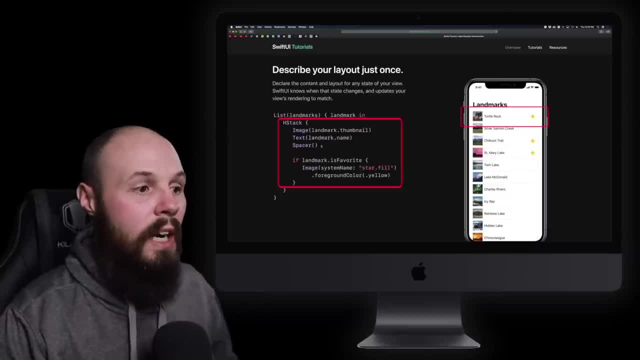 the spacer is the space in between turtle rock and the star, and then you can see- here is an if statement- that hey, if the landmark is marked as a favorite, then show the star. so you build this h stack, which is a view of horizontally stacked other views. 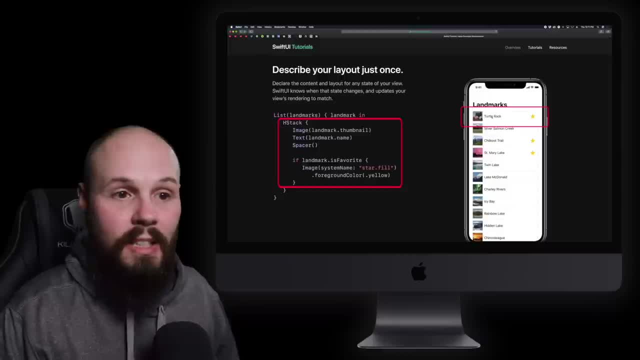 so again, the horizontal stack is the image on the left, the text right. next to the image put a spacer and then have the star on the right if it's marked a favorite, and then all the table view is is a list of those views. so this whole table view is built in just this little bit of code. 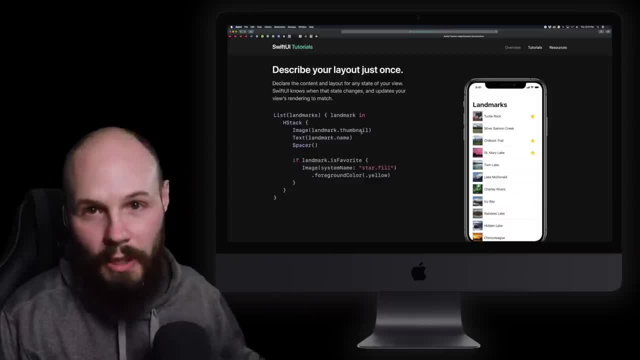 of course, except for the data right, like landmarkthumbnail, like all that code is in you know a data model somewhere, but the actual ui code for the table view like this is it? like? it's actually pretty amazing and, like i said, we're going to build one, uh, in the next video. simplify: 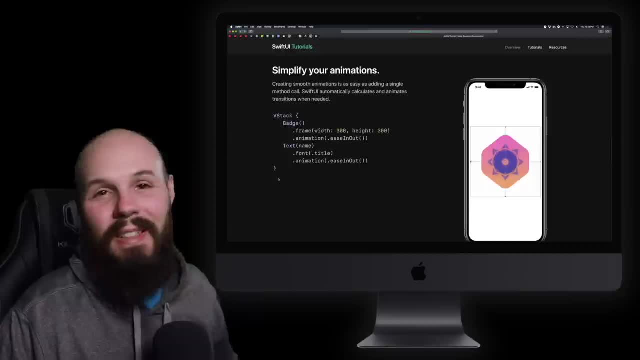 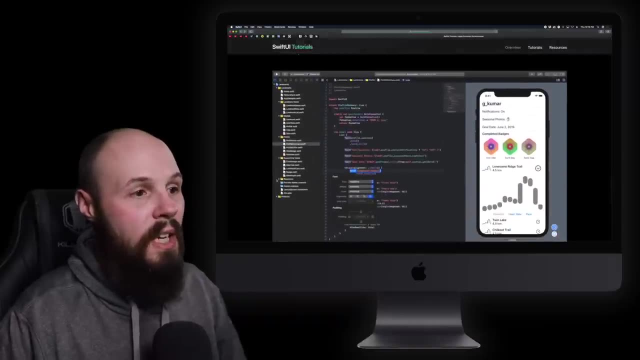 your animations. um, we're not going to see this in the example again, it's not a huge, thorough tutorial. animations are super, super easy. uh, in swift ui as well. and then you saw this: uh, the x code. uh, you see it live. uh, what they mean by live? is you remember when we were building like our, our? 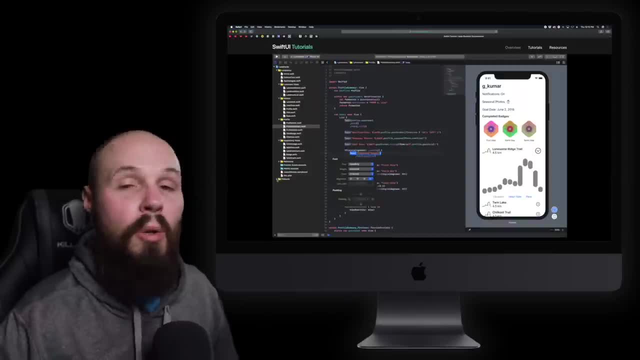 other apps. if we wanted to see the changes, we had to run it. okay, pull up the simulator. cool, now we play with it. well, as you're making changes, the canvas updates live and even if you're running your app and you change the title like, it updates live. and again we'll see that in action in the 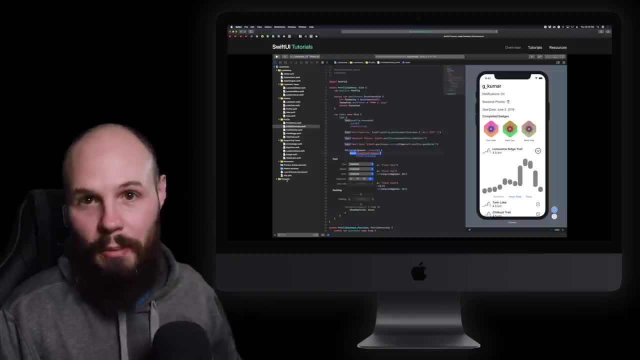 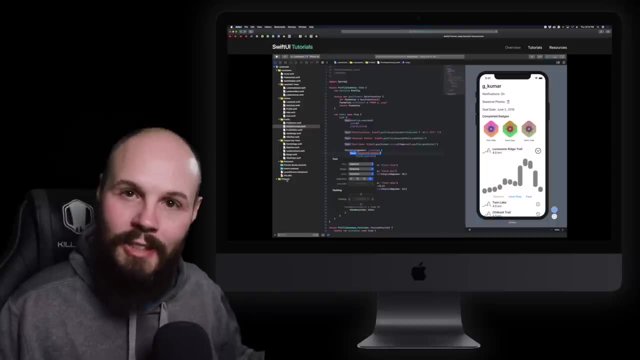 next video. but that is a great productivity win for development. right, because you remember what it was like. right, we would make a change. all right, let's run it. oh, that was broke. okay, make the change, run it again. that takes a long time. all right, keep it moving. um, okay, this is other stuff. 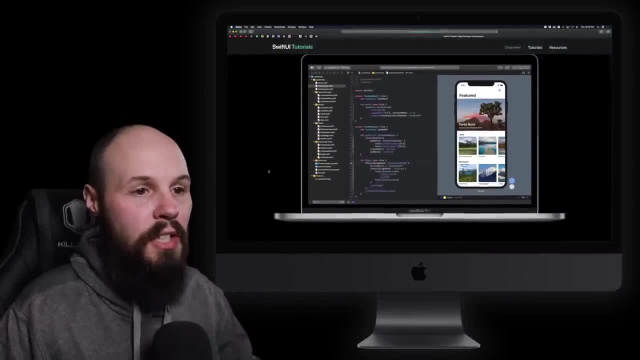 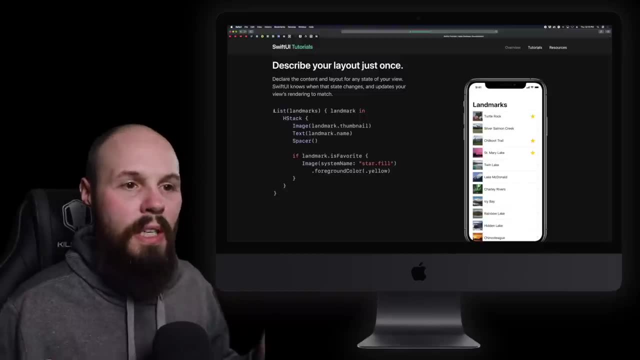 but, yeah, i highly recommend checking out this page. um, and the great thing that i forgot to mention is when you use these uh elements like this list, the reason it is a list and it is kind of, you know, generic, if you will- is because when you make a list like this, it translates that into whatever. 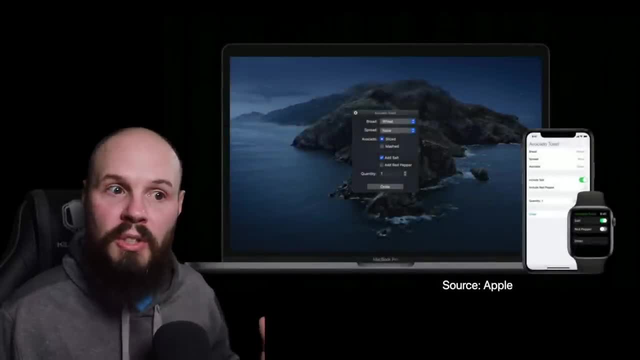 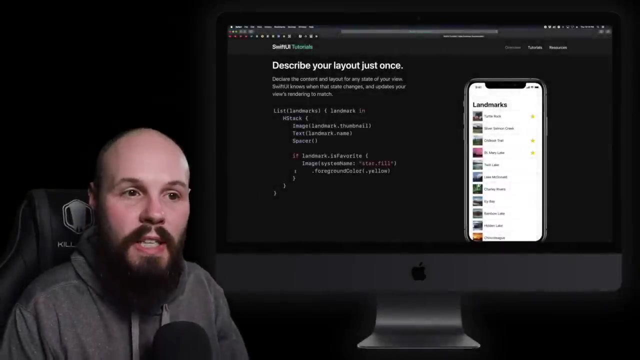 platform you're on. so, for example, a list on a watch looks a lot different than this list, but it's going to adapt for you, right? so by using swift ui, it goes across all the apple platforms, right? mac os, watch os. so, uh, it's a great way to kind of write the code once and then you know. 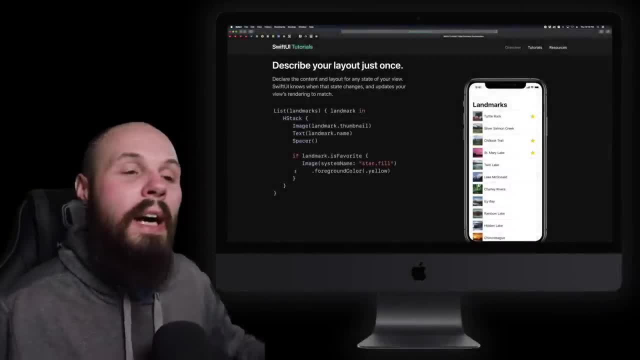 you get all those other layouts. you don't have to create a full-blown, separate mac app again. that is high level. if you're converting an ios app to a mac app, there is some stuff you need to do. of course, i'm not just saying it automatically transfers, but building in swift ui does a lot of the heavy. 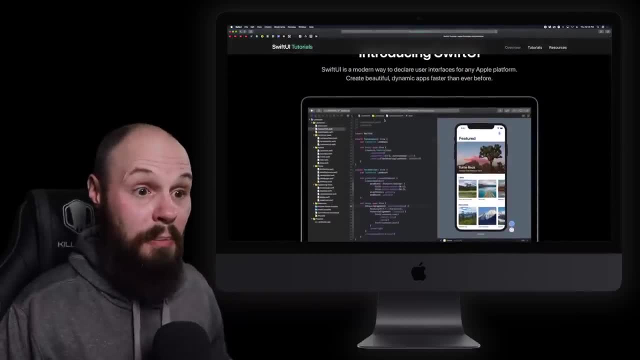 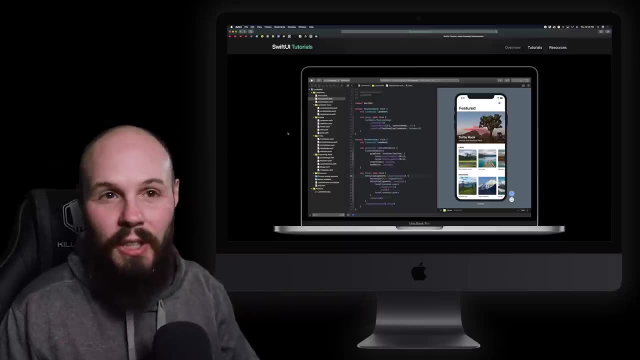 lifting for you. so, to reiterate, before we move on to uh, actually building something in swift ui, we're still very early. i know it's exciting to want to go learn swift ui, um, but as a beginner, you're going to be much better off learning ui kit first, because swift ui is still so, so early. 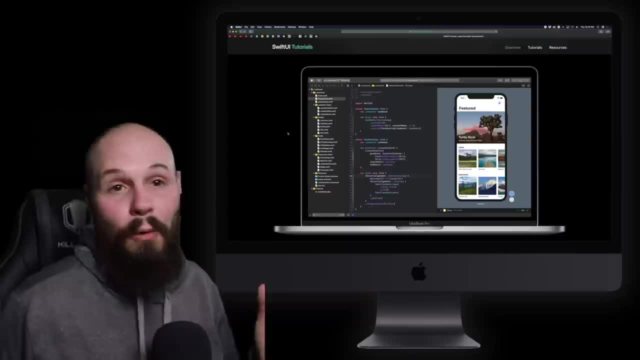 so nascent that things are going to change rapidly, like i don't know what's coming at wwdc in a couple months. but i'm expecting some big changes for swift ui, just like there was from swift 1 to swift 2 and swift 2 to swift 3.. like, swift changed a lot during that time period. 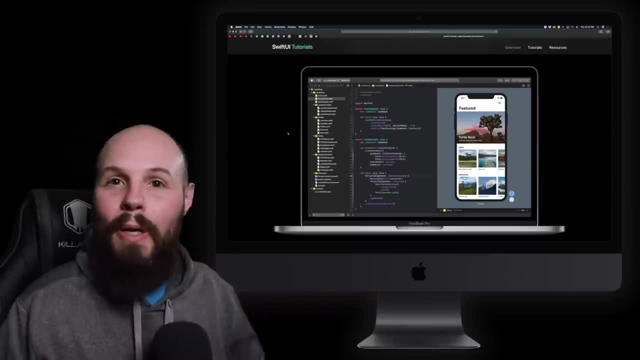 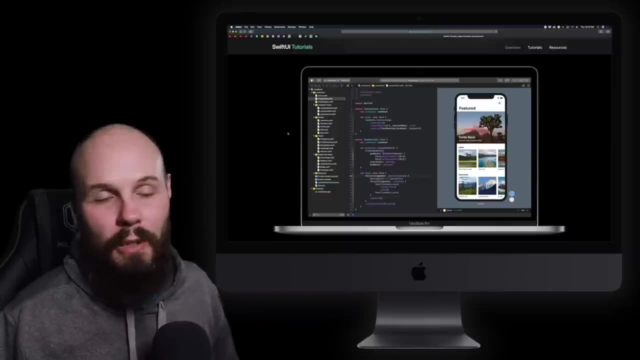 we're all expecting the same to happen with swift ui. so again, my recommendation is: let us sort out swift ui first and then kind of come over and learn it, but definitely like take some time to play around with it. again, my one big advice: don't split your time. 50: 50 right. 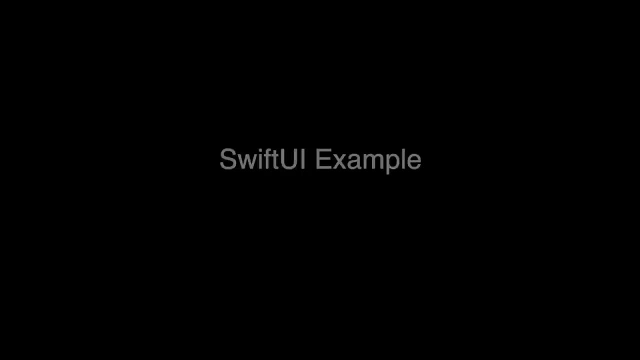 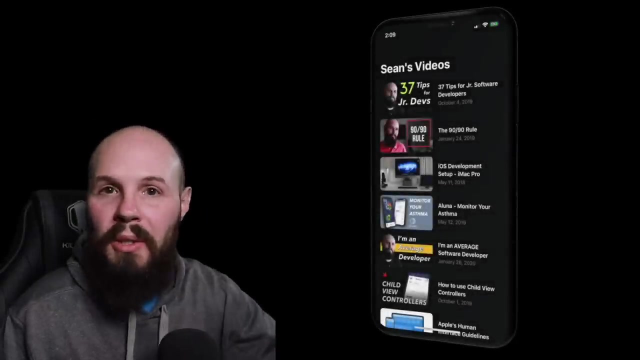 focus on ui kit first. that's what i would do if i was starting right now in this swift ui preview. we're going to build this table view which has my thumbnails and the youtube video title and the date it was uploaded, and it's going to be in a table view. 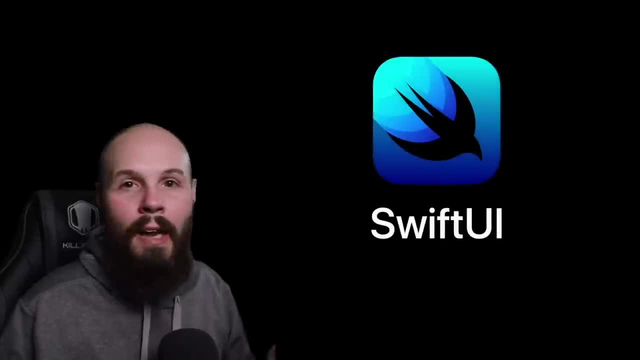 i'm going to show you how to build that in swift ui. now, again, i stress, swift ui preview, not swift ui beginner tutorial. um, because again i know i've said this before, but i will reiterate: uh, explaining all the the basics of swift ui, like that would be 10, 15 more videos, like that's an. 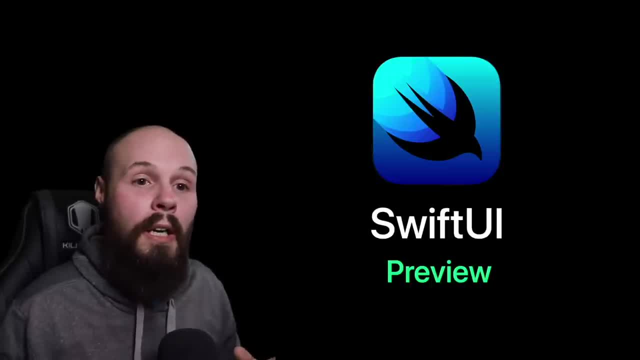 entire other course. good news: i plan on uh releasing that course by the end of 2020.. why so long? why the end of the year? because it is april of 2020 right now. well, like i said in the previous video, i'm expecting big changes at wwdc this summer. 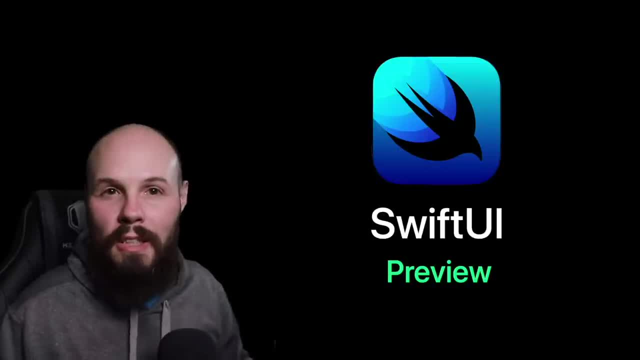 uh, and then it's got to go through beta and won't be officially released until fall of 2020. so that is why the end of the year, the swift ui course will come out. so if you're super interested in swift ui, uh, stay tuned for that. but this is just a preview because, again, the whole point of 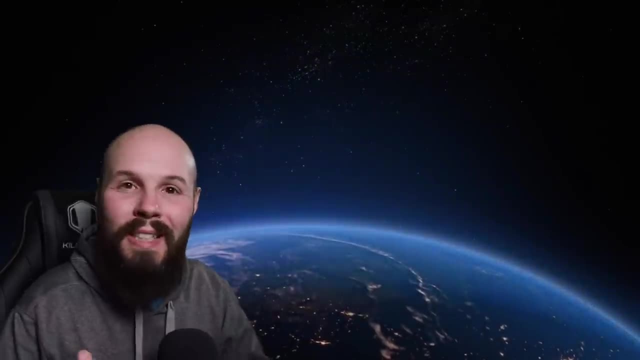 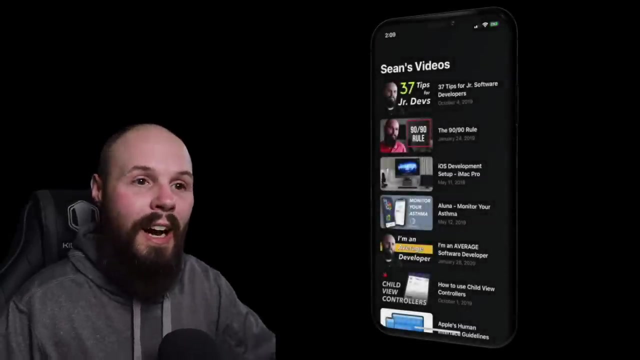 this course was just to expose you to the whole world and and show you what exists and give you the high level concepts. right, but you will be able to follow along and type along with me and have this end result. i just may not stop and break down every little super basic thing. so again, feel free. 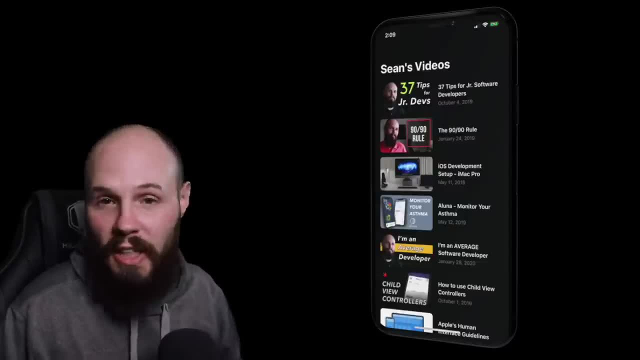 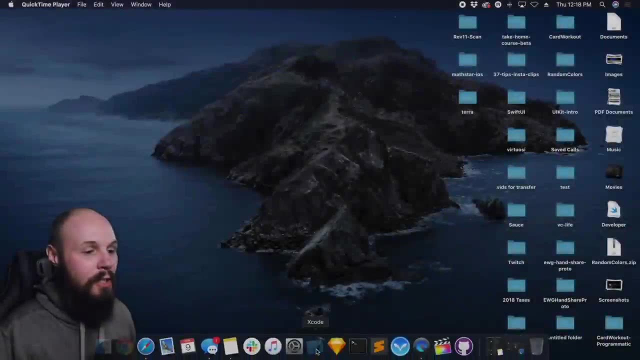 to follow along, but this is not meant to be a comprehensive. you understand every aspect of swift video. all right, that disclaimer out of the way, let's get started. here we go: uh, open up xcode new project. uh, something's gonna be different now. single view app: that's fine now, uh, we're. 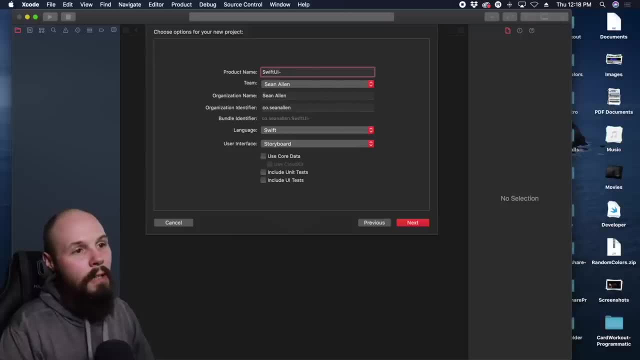 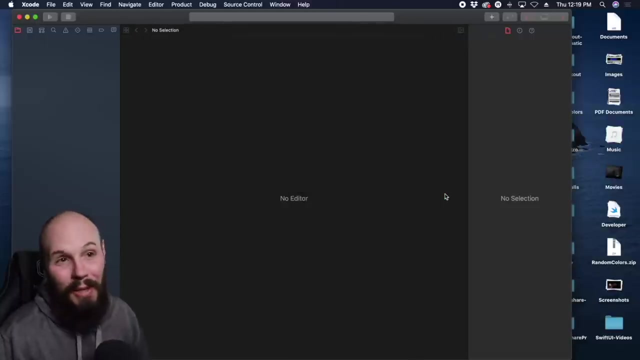 gonna call this swift ui. uh, videos, that's what i'm gonna call it, and sean allen. sean allen, put your information in there. as always, language is swift. here's the big deal, not storyboard. swift ui- there we go hit next create. oh, i guess one thing might be a little too late now. uh, swift ui does require xcode 11 and mac os catalina. 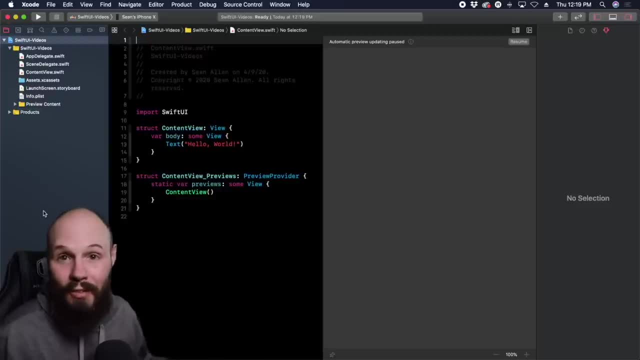 so if you're not on mac os catalina, or you're not on xcode 11, um, just watch the video. you can't type along. uh, so that is the one of the downsides is also, you know, focusing on swift ui is that it requires all the latest and greatest equipment and if somebody wants to use your app, that uses. 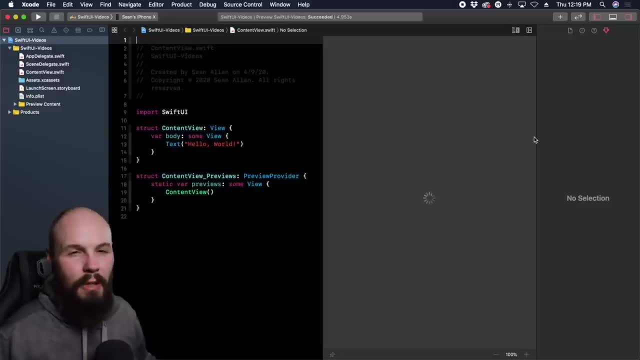 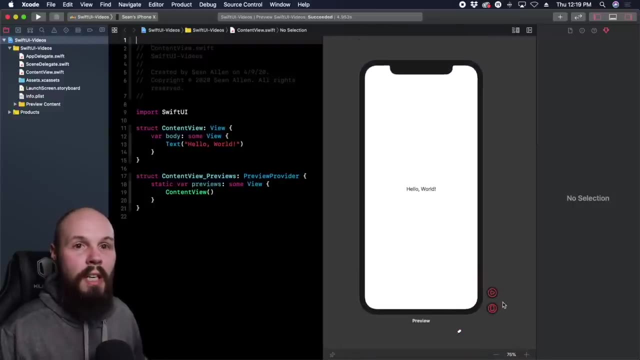 swift ui. they have to be on ios 13, which might not be that big of a deal, but disclaimers nonetheless. all right, my canvas is loading up awfully big. let's minimize it. let's actually minimize this right pane. we're not going to need. 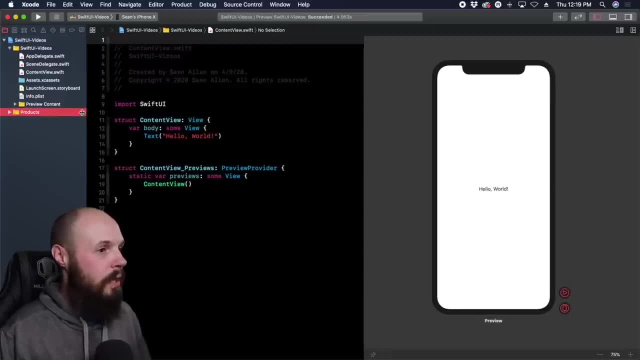 that again, i want to make sure my environment is good. okay, so here we are. as you can see, hello world. i'm going to click on that and you see it automatically highlighted the code here on line 13, and put a nice little red box around that you'll notice. there's no constraints, there's no label. 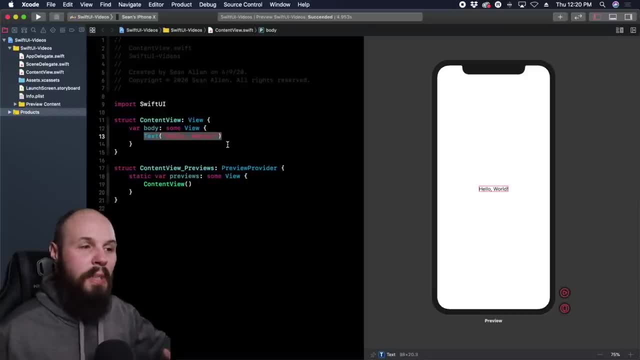 right, it just knows where to put it now to start building this up piece by piece. instead of hello world, let's put in uh video title, so you can see what that is. uh, this is what we're going to start building now. below it, as you saw on the design, here, you know we have our video title and then 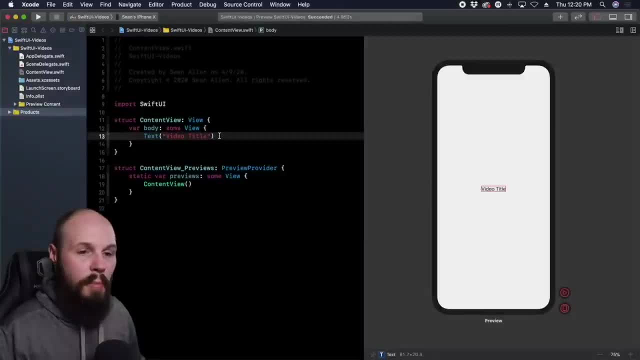 we have the date below it, so we're going to need another text, uh, right below it. so two options here. uh, we're going to do it the quick way, and then i'll show you how you can do it just by typing it out too. so remember, i said earlier you can do a lot of stuff on the canvas, and it'll put the 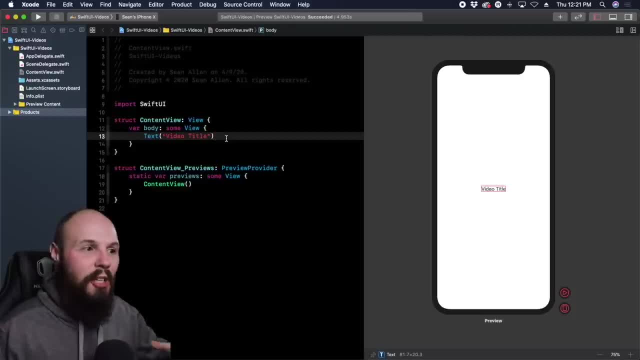 code in automatically. that is how you may want to start out, because that is how you're going to learn, um, basically how swift ui is working, what the modifiers are. but once you have done swift ui for a while and you have things memorized, you're probably going to be a lot faster typing, so just 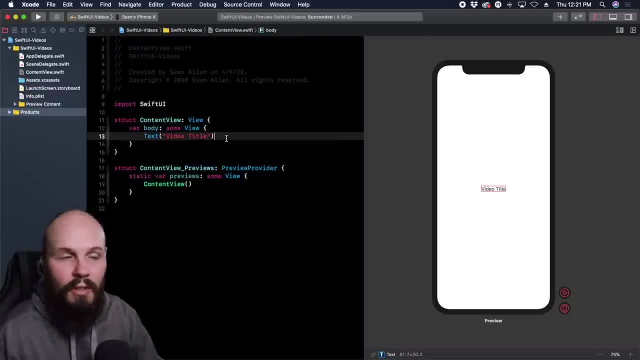 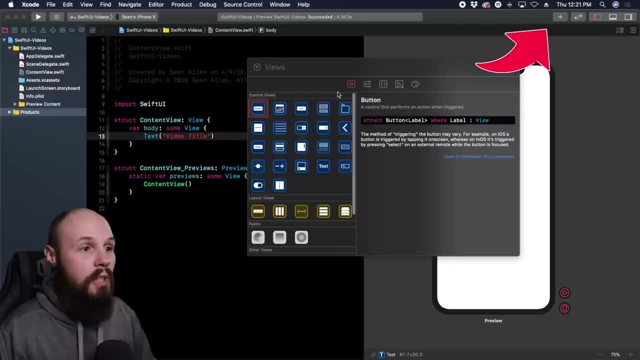 know that that's probably going to be your evolution of using swift ui: start on the canvas and then eventually shift over to typing. so we're going to start with the canvas, just like on storyboard. hit the plus button up here and you can see. you have a whole list of stuff here, so let's. 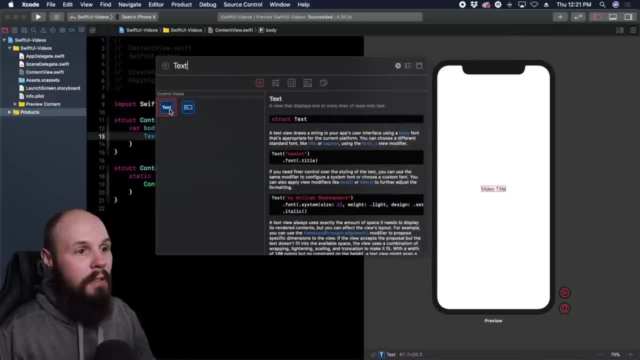 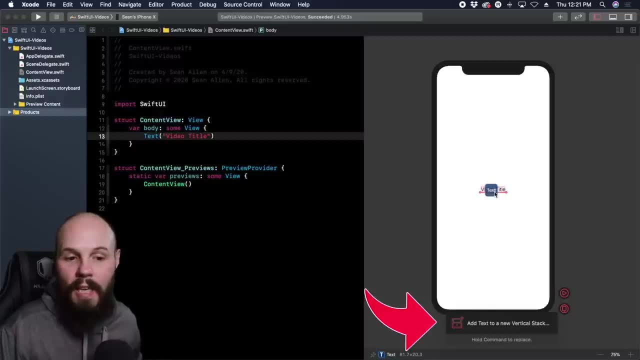 type in text. that's what we want. so if i drag text onto here and you can see, hold the button and you can see like a solid red line and look right below my canvas here, add text in a new vertical stack. if i move it to the left, add text in a new. 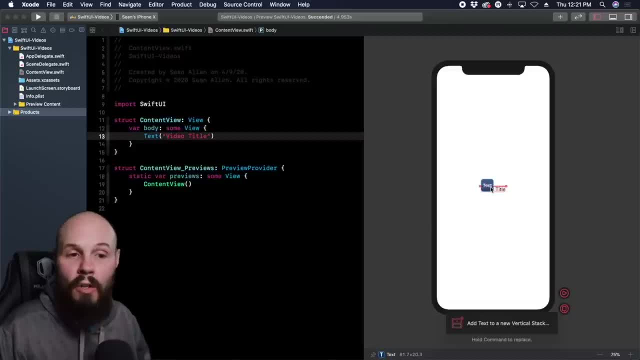 horizontal stack. same thing above it. add text to a new vertical stack. so a big thing with swift ui is v stacks and h stacks and z stacks. so v stack is a vertical stack, an h stack is a horizontal stack, like i explained in the previous video how their cell was horizontal, and a z stack is like 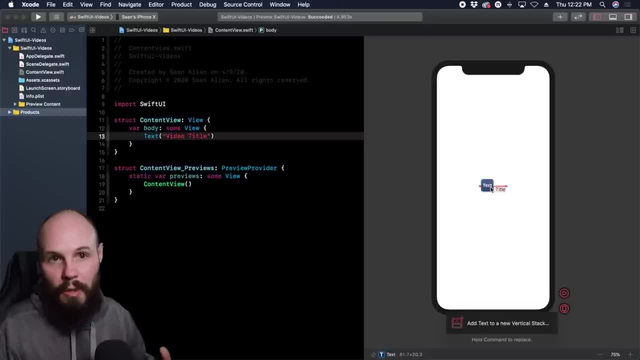 layers on top of each other right, not not to the left of it or to the bottom of it, like right on top of it. that's the z stack and then you can see that it's a vertical stack. and then you can see that it's a z stack. so we want to add this to a vertical stack right below it, so you can see how. 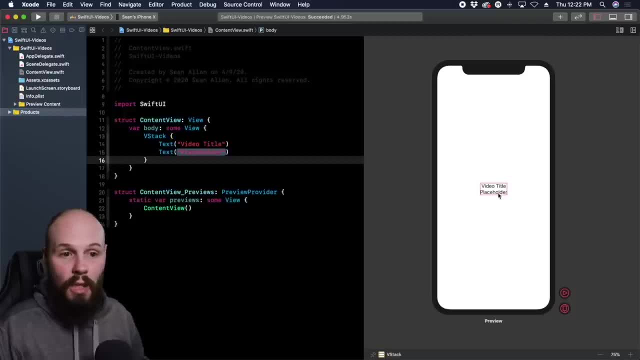 you have this solid red line here, let go, and you're going to get the text below it- see placeholder. now look what it did to my code. it added the text here and it automatically wrapped my two labels in a v stack, right, all by just dropping that onto the canvas. it fills in the code, like i said. 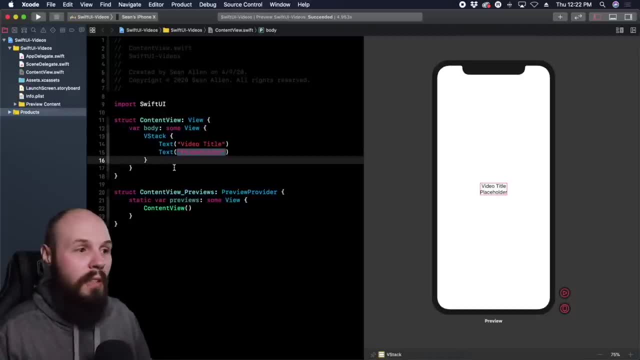 um, now, now you can kind of see like if you already knew you wanted a v stack with two labels in it, you probably could have typed this out faster than like dragging it and dropping it. so hopefully that illustrates what i'm talking about. and then you can see that it's a v stack and it's a z stack. 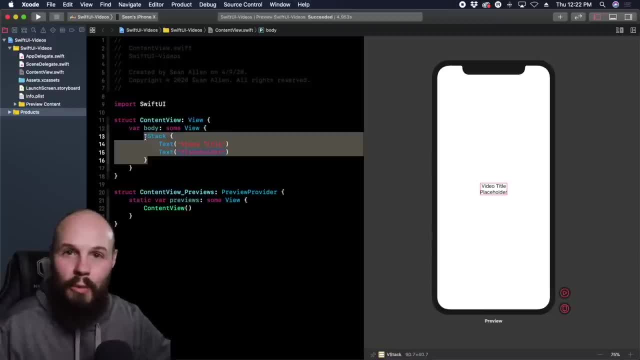 about is: you may start off on the canvas, but as you get better with swift ui, you'll migrate to actually just typing it. so we don't want this to say placeholder, uh. we want this to say: uh, date uploaded, right, okay, um, now let's look here they are. um, they're kind of close here, like right. 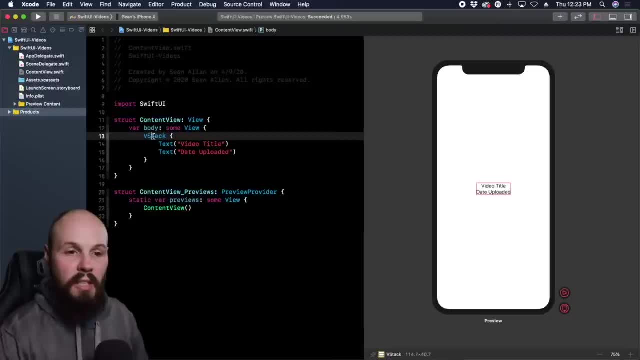 they're kind of squished together. but if i click on this v stack you can see. so the v stack is only going to fill up as much space as it needs. so that introduces me to the concept of a spacer. so i'm going to go ahead and create a space here. and i'm going to go ahead and create a space here. 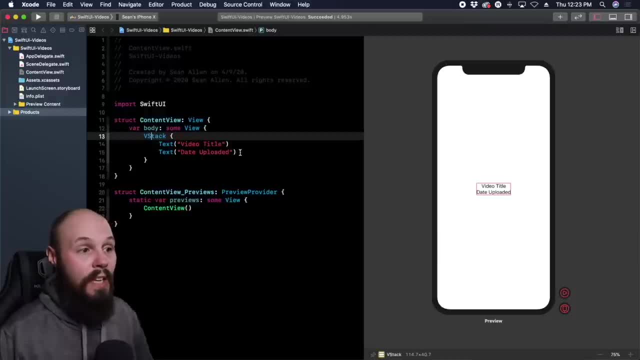 so i'm going to go ahead and create a space here and i'm going to go ahead and create a space here. spacer will fill up like the rest of the space. so if in this v stack i type a spacer down here, watch what happens. it shoves everything up to the top. because what you're looking at in this v stack 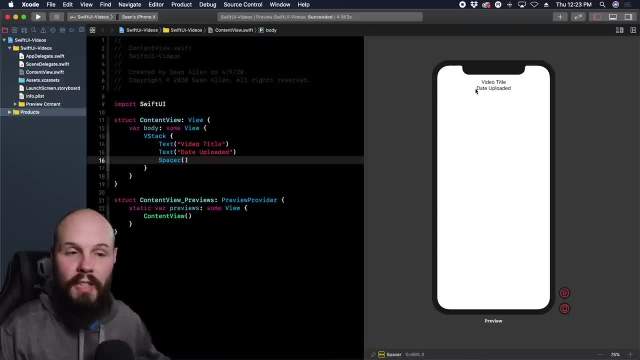 is you have one text label at the top, another text for date uploaded and then the rest of all this space on the phone is the spacer right? so same thing. if i put the spacer in between the text now, look boom, it split it up top and bottom. so again the v stacks fill up the entire, not 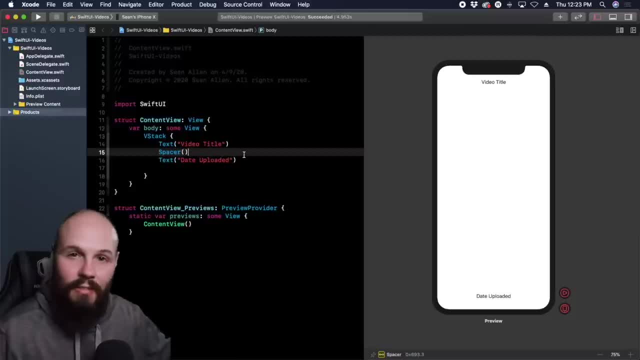 necessarily the entire phone on the phone, but the entire space on the phone and then the rest of all the time, because again you can have v stacks inside of v stacks inside of an h stack, like there's layers to this stuff, um. but that is the basics of what like a spacer does. now we can add: 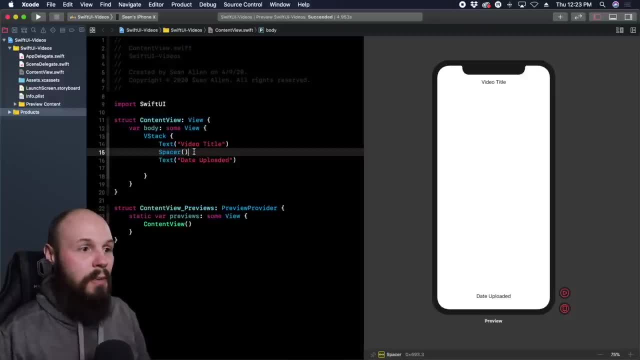 a modifier to the spacer. oh, we're getting crazy. um, so let's do that here. we can do dot, frame, and then you can see we can give it a whole frame. width, height, whatever, we just want to give it a height. so i can actually like delete all these other ones and the frame of my spacer i want to. 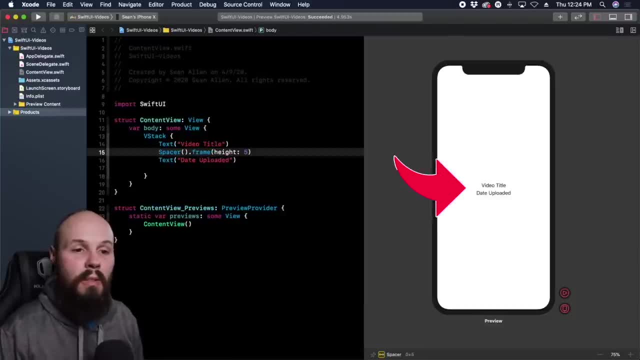 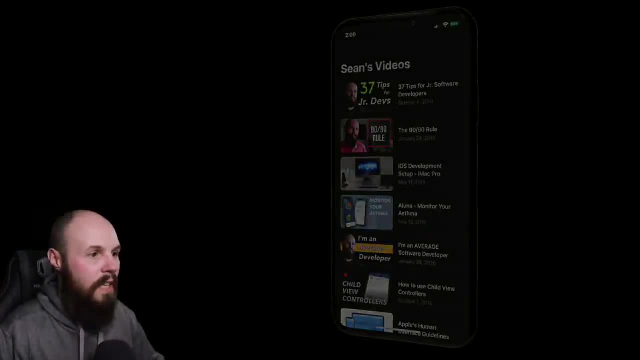 do that right. so you see, now i just added a little bit of space in between video title and date uploaded. now you may notice, in our design those are aligned left. those aren't, um you know, centered like they are right now. so if i click on my v stack- and here's the cool thing, if you command, 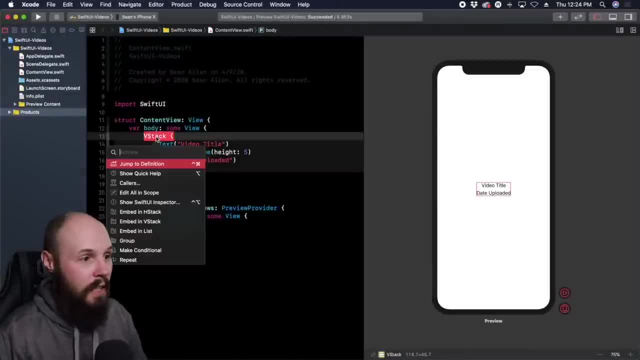 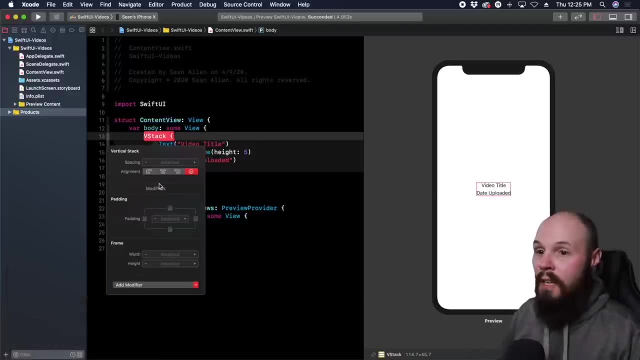 click on your v stack and you can do this in code: watch i command, click. i get this menu and hit show swift ui inspector. like this is the cool thing, you're going to get all this stuff right. so alignment, like we want this to be a line left, so let's click on that alignment and look. look at my. 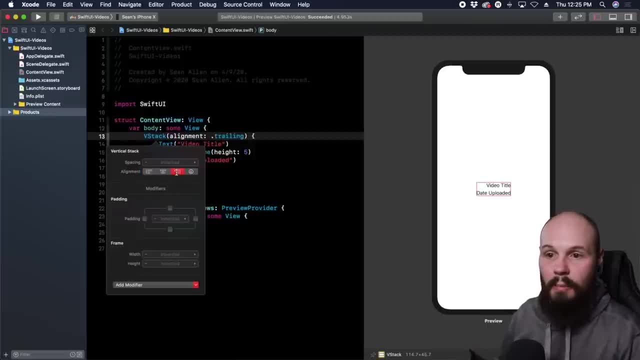 canvas, they align left instead of center. so i'm going to click on that alignment and look, look at centered. watch, i'm going to hit them: align right. bam, they aligned right, centered, centered, cool. and then, like i said, this is when you can start learning your modifiers, right. so here's the frame. 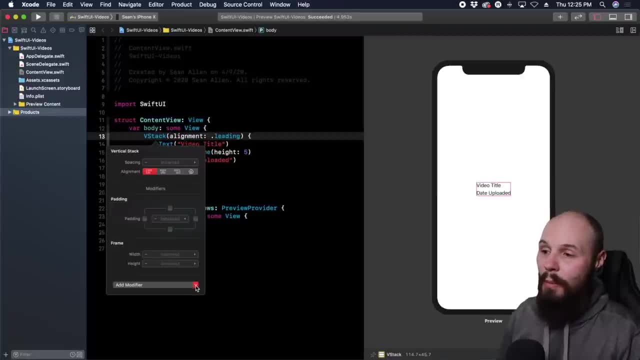 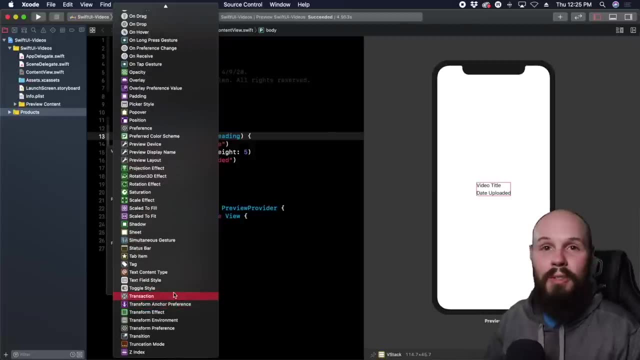 padding, uh, and you can add modifier. now watch what happens when i click this. it gets crazy, you can see. look at all the. there it goes. i was hoping it got big like that. look at all these modifiers. so this is what i was talking about: how, using the, the canvas, to help you learn these. you 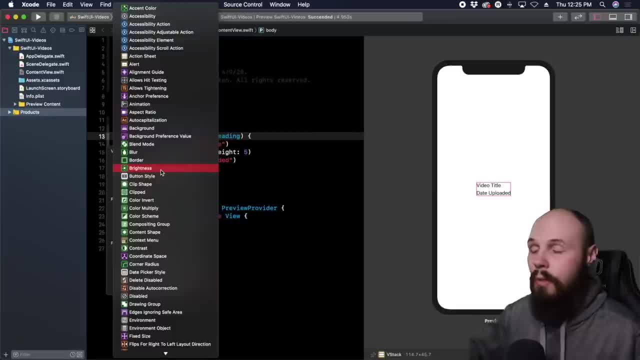 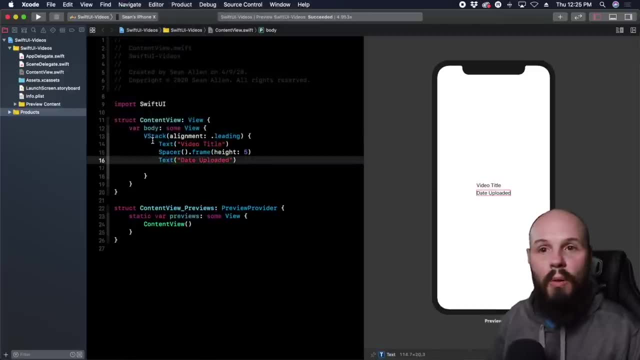 know before. you have all these like memorized, but once you have memorized, like i said, you can just type it out real quick. so these are all the different modifiers. uh, you can do. we're not going to add a modifier to this just yet. we just wanted to make sure our v-stack was leading aligned. 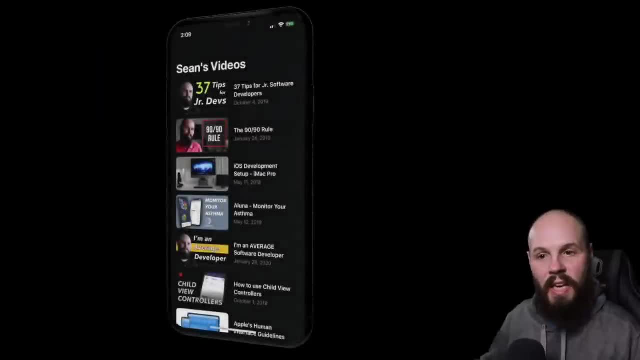 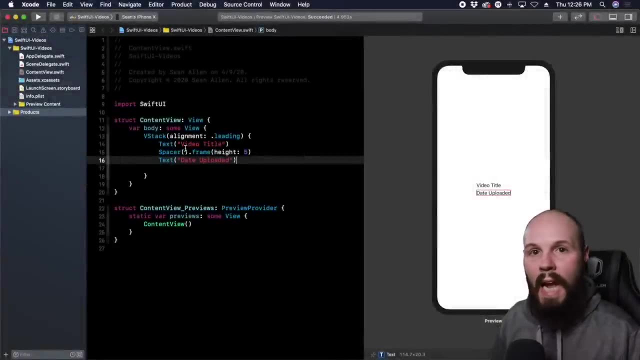 so they align left. next, we want to add our image again. if you look at the design, the thumbnail image is to the left of our date and title, so our title and date are in a v-stack by themselves. however, we want to put the picture to the left, so that would be an h-stack right, the left side of. 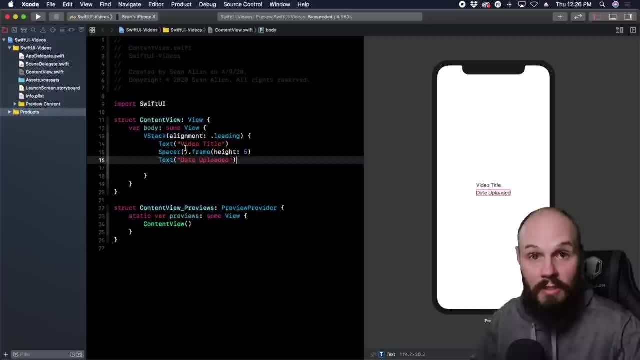 the h-stack is my image. the right side of the h-stack is the v-stack that holds my my title and date uploaded. so remember i said you can have h-stacks inside of v-stacks. inside of h-stacks, like again, there's levels, but if you just picture, 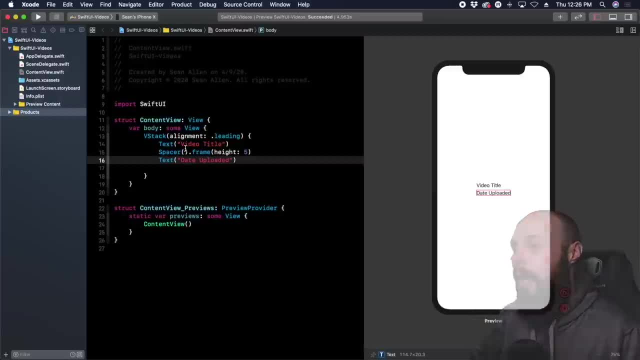 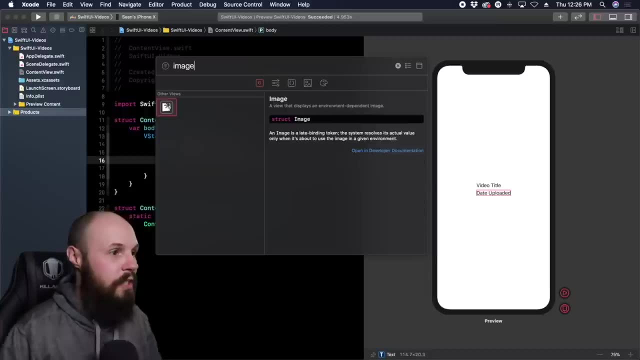 the boxes, um, and the items in the boxes. that should help you out. so we want to add an image, so hit the plus button type: uh, image. oh, i gotta spell it right- image, okay, again. drag it onto your canvas. now again, we can add it in a vertical stack. that's not what we want to do, right we? 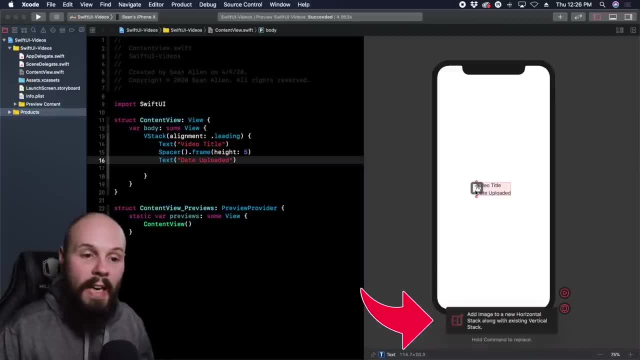 want to put it on the left and you see, you get that solid red line and it'll say: add image to a new horizontal stack, uh, along the existing vertical stack right. it tells you exactly what's going to happen. so we drop the image there. well, there is no image because we don't have an image name. okay, uh, let's. 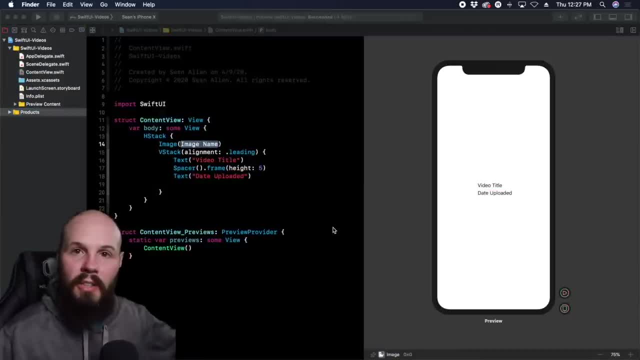 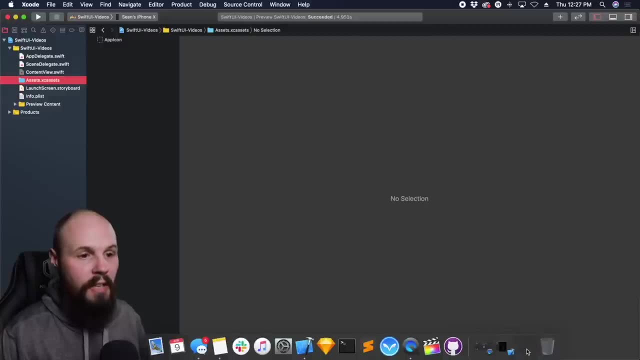 actually upload our images now. so i have these prepared, but i'm going to link to these images in the description so you can download them. but, just like before, click on your assets folder, uh, go to your finder that has the images. here's my. here's 12 thumbnails of mine i'm going to drag. 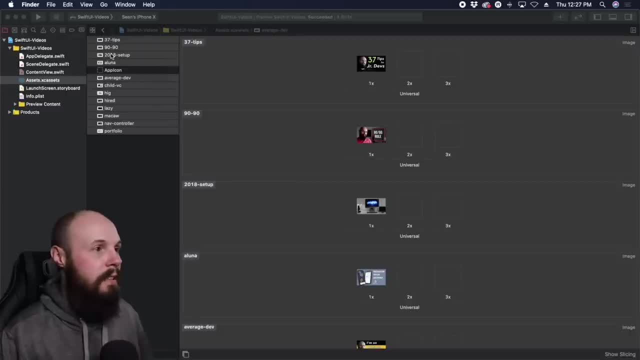 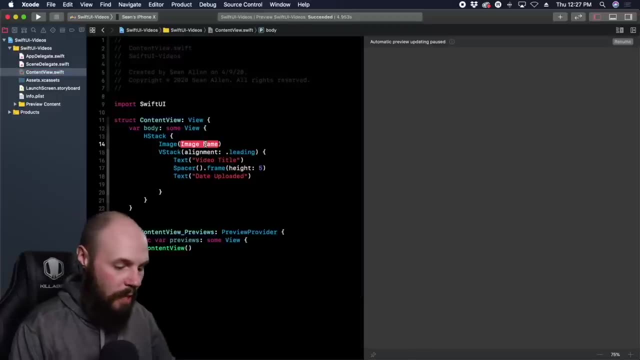 them in here. cool, and we'll pick 90: 90 as our first. you see the name here. let me click on it: 90 90, that'll be the name of our image. so go back to the content view image name: 90-90. um, sometimes, uh, your automatic preview will get paused. uh, if you just hit resume, that'll. 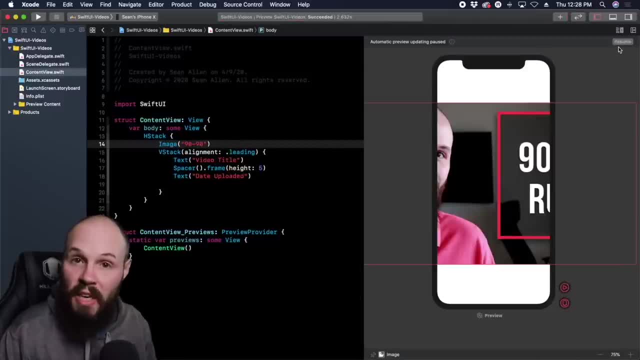 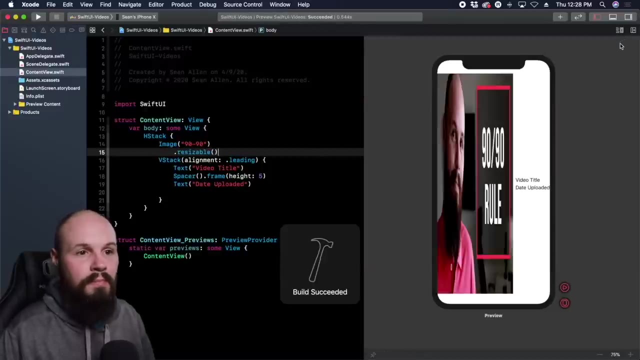 pop back up. okay, uh, not the desired effect. huh, our image is huge, so to make our image fit, we want to give it a modifier. we want to give it the resizable modifier so you can do image dot resizable and watch this update here. well, maybe hit resume. okay, still not the desired effect. what that did was that. 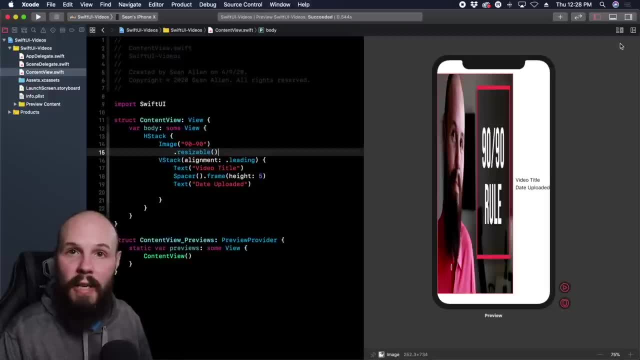 our hdac right. you see, the right side of our hdac is still our title and our date uploaded. the left side of our hdac is the giant picture, but it did squeeze it so it only fit on the left side. so what we want to tell it to do now is to keep the same aspect ratio right, it's a 16 by 9, uh. 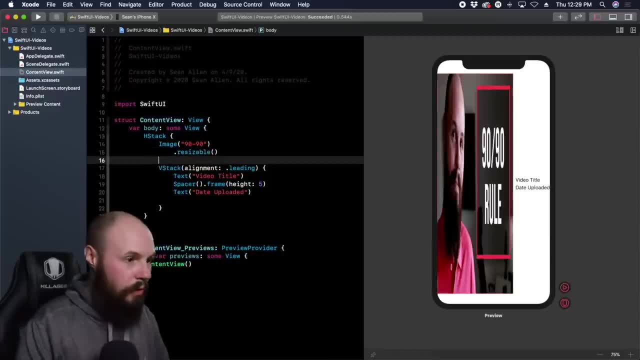 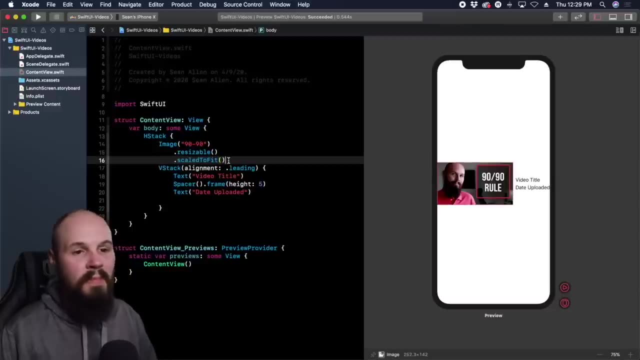 make sure you keep the same aspect ratio and that'll make it look better. and to do that, we can do dot scaled, uh, to fit scales the view, to fit its parent. bam, we keep our aspect ratio there. um, our image is a little big, so we're going to do that, and we're going to do that and we're going to. 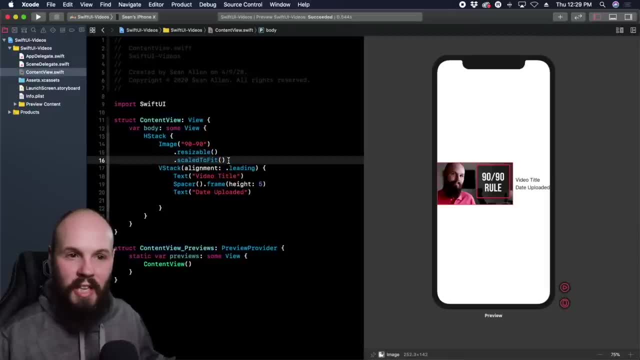 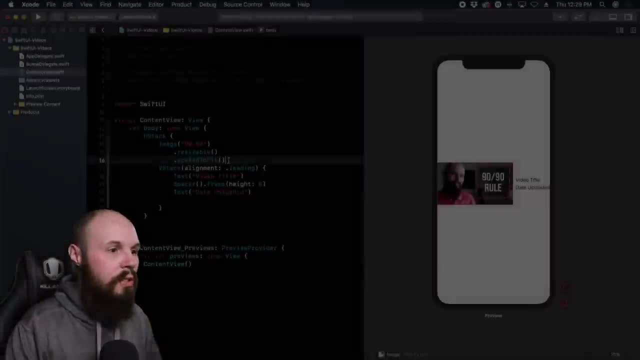 do the same thing. right, it dominates the, the whole hdac, right, it's taken up like 60 of it. and again, if you look at our design, uh, it's not, you know, it's smaller. so what we can do here is also assign a frame to the image. now you see me typing code, like i'm just kind of used to that, but again, 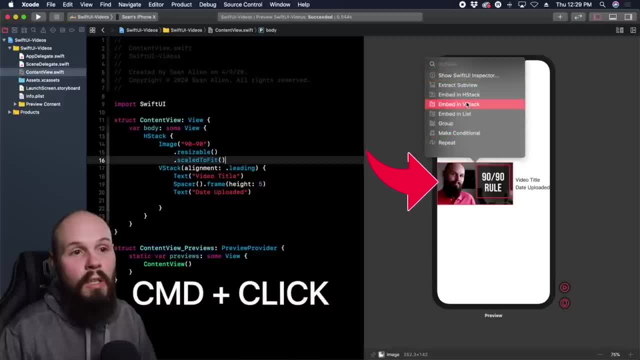 what i can do is if i command, click on the 90- 90 rule, uh image and say: show swift ui inspector, you can see i can do my modifiers from here as well. so, frame, i want to give a height, i want to give a height of 90, so i do that and i hit return. 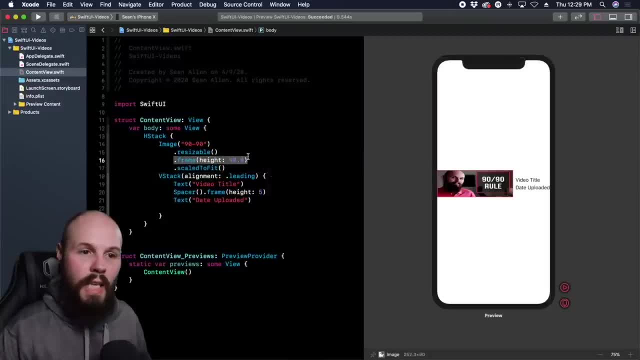 it gave me a frame of 90 here, right on line 16, and here you notice that's still not what we want. so, uh, order matters. this is kind of the biggest learning curve, um, with swift ui. these are all called modifiers, by the way. what you can put on there and the order of your modifiers matter so 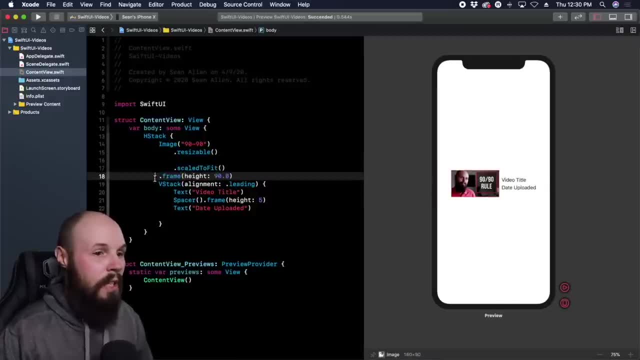 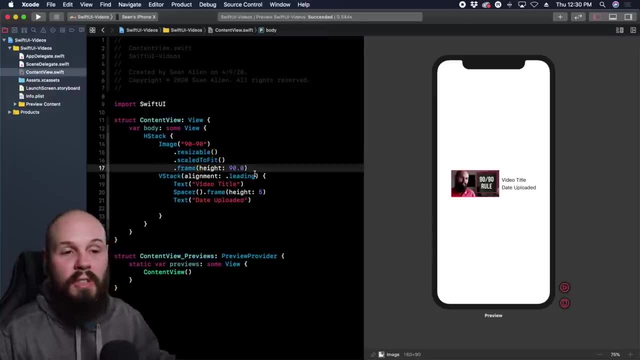 uh, you're going to see, sometimes you just put some things in the wrong order and that doesn't give you the behavior you want. so, like i said, i put the frame before scale to fit and that didn't give me the behavior after scale to fit. now that's starting to look a little more like what we want. 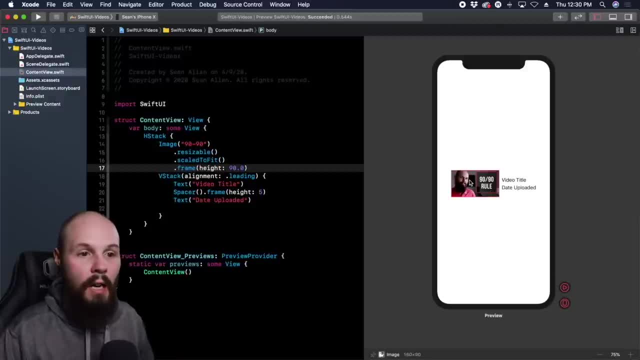 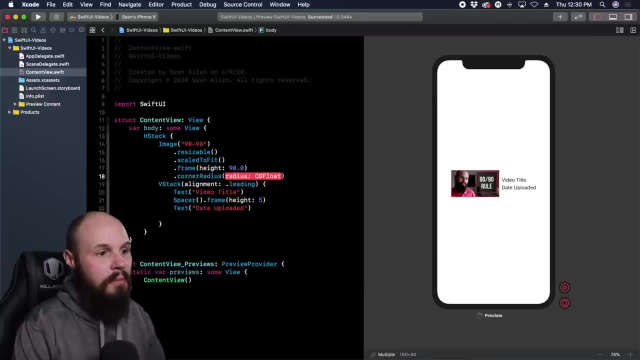 and the last thing we're missing from this is the corner radius. so again, uh, command, click on the picture, there's. there's tons of different ways, right, i could just type. i could just type dot corner radius right, and then of eight, bam, like i said, once you know it, typing, it is going to be so. 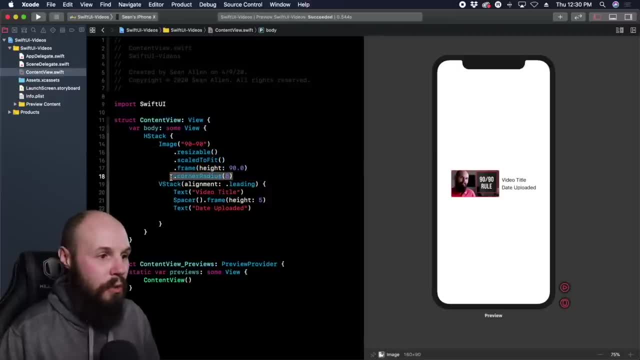 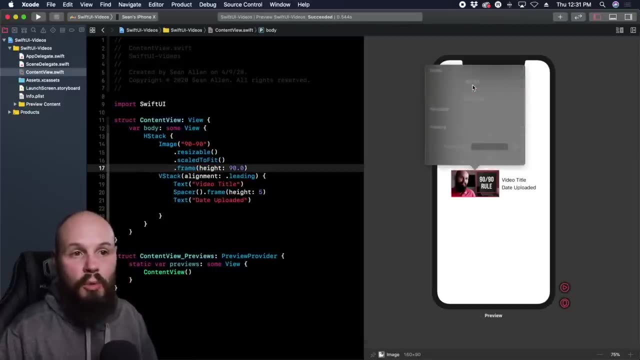 much quicker. but because you're a beginner, i want to show you. let me delete corner radius. i want to show you how to use the canvas because that's how you're going to learn and memorize all these modifiers. so hit show swift ui inspector. you can scroll down add modifier. you see our whole list of. 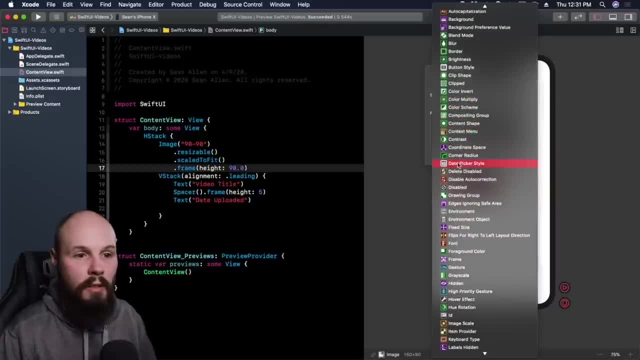 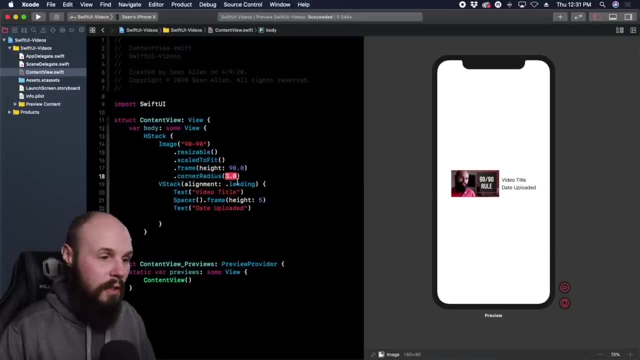 the modifiers. uh, right, and then we're going to look for corner radius. that's what we're looking for here. okay, cool, corner radius, let's add that. and you saw here, uh, it gave me, it gave me the code. right, it spit the code in here. it defaulted, defaulted to three. we're going to make it eight. 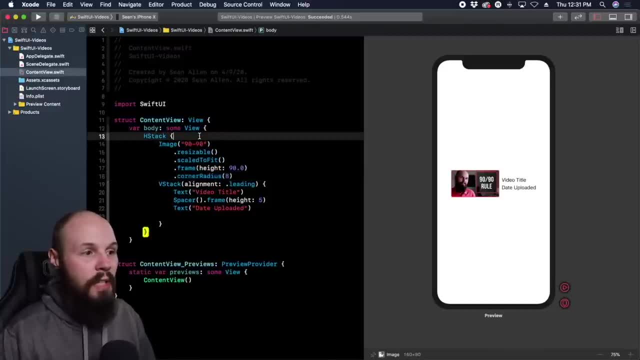 uh, that's what the design wanted. so now our image here is looking- let me kind of click off this so it doesn't highlight in red. uh, it's looking kind of like what we want. um, one thing i'm noticing here is the first is our video and title in our image are just squeezed a little bit too close. 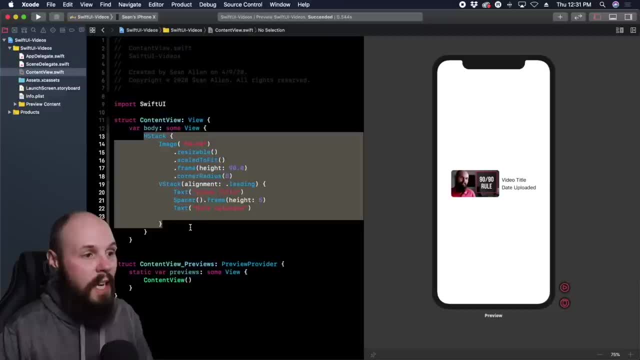 together. so let's put a screen here, and we're going to put a screen here and we're going to put a spacer in between them, right? so you see our h stack here. uh, so you see, the image is on the left side of the h stack and then our v stack is on the right. well, in between them, let's add a spacer. 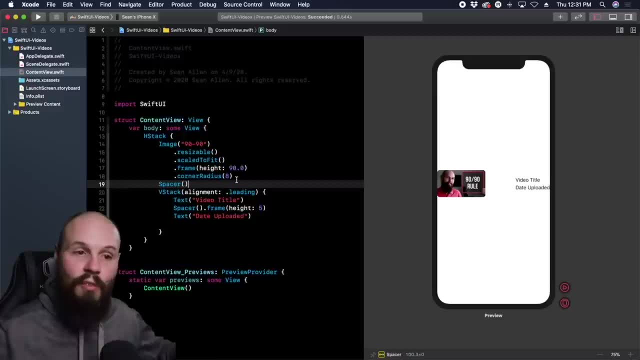 and okay, remember this, remember the- the view fills up the whole screen. well, you see, by putting a spacer in the middle, it pushed the text all the way to the right and the image all the way to the left. so that's not quite what we want either. so again, remember how i gave the, the spacer down here. 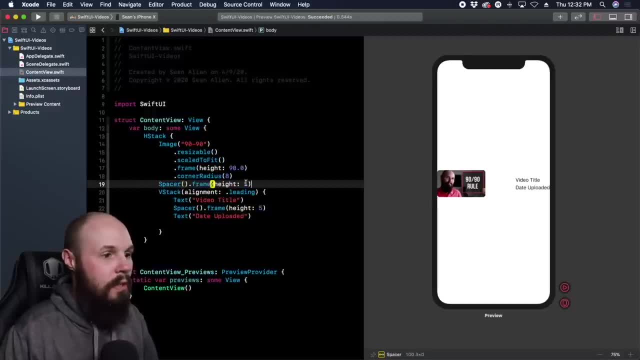 a frame. well, i can do the same thing, so i'm just going to command v, or copy and paste that, and not a height. we don't want a height on the spacer, we want a width right, because we're in the horizontal- uh- stack. so let's make the width 16 again. this is just based on design. okay, so that's. 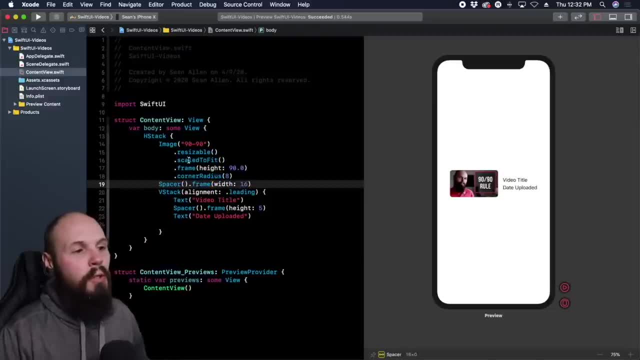 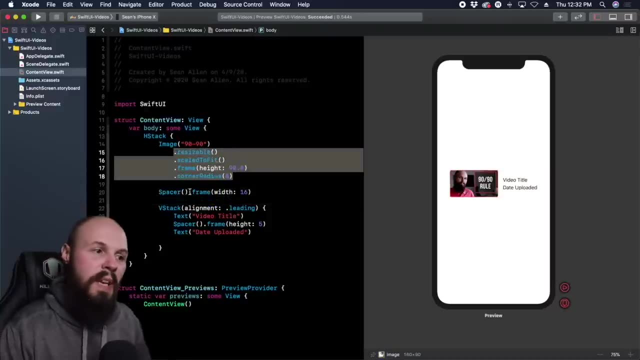 good, proper spacing, uh, that i want now to avoid confusion. you may notice how i'm just typing this list of modifiers here and it's like a vertical stacking list, right like this, and. but on the spacer i just did dot frame. so if i only have one thing i'm adding to the spacer, i like to put it: 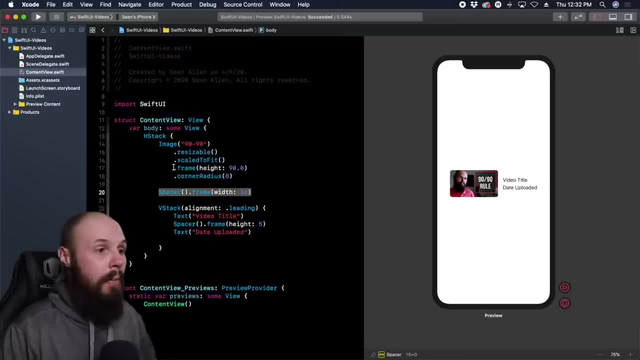 on one line, and this is pure stylistic choice, by the way. um, however, obviously, if you have a, you know four of them. it makes sense to put it on multiple lines rather than doing like image dot, resizable dot scale to fit dot frame like all on one line. that becomes very hard to read. 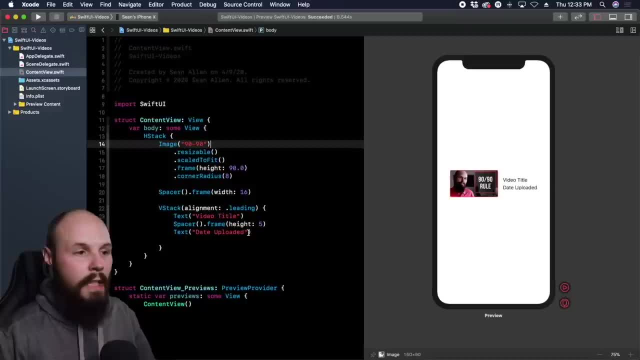 um. so again, if i only have one thing, i like to put it on one line. now let's play around with the text here. instead of video title, let's actually put the name of this so say: uh, the 90: 90 rule. and i'm testing, um, like how how this label works. so the 90: 90 rule is a great rule. um, i'm seeing how this. 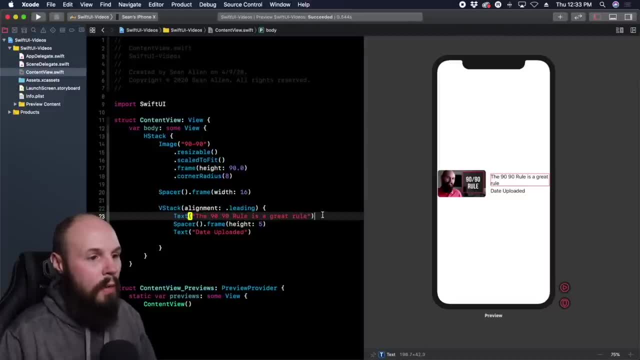 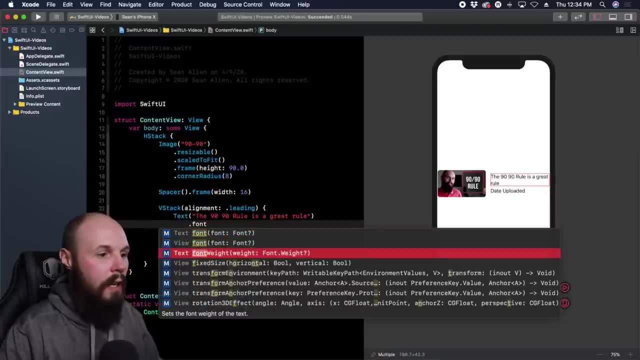 works. you see how it's spaced out here and i'm seeing how it's spaced out here and i'm seeing, and gave me a live update: um, let's add some modifiers to this text. so this is our title, so let's give it a font weight. so, as you can imagine, there is a dot font weight, uh, modifier here. and 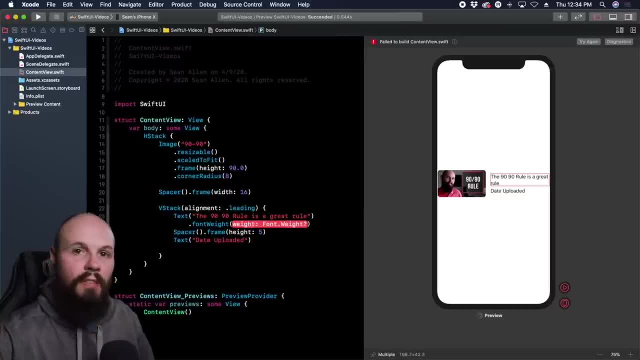 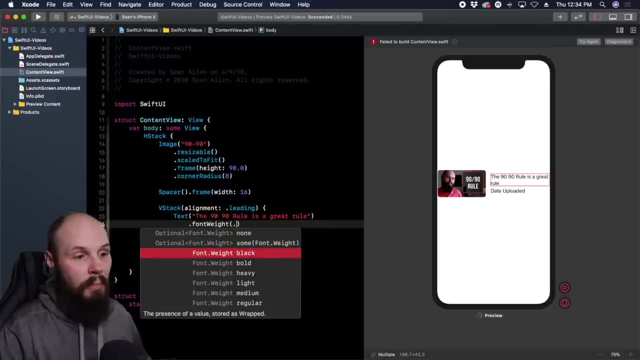 again, you can do the same thing. you could click on your uh, your canvas, find the modifier, drag it onto the canvas. um, again, i'm just quicker typing, kind of the habit. so again, if you hit dot, here's your font: weights, bold, heavy. you know whatever we're going to do: semi bold uh for this title. 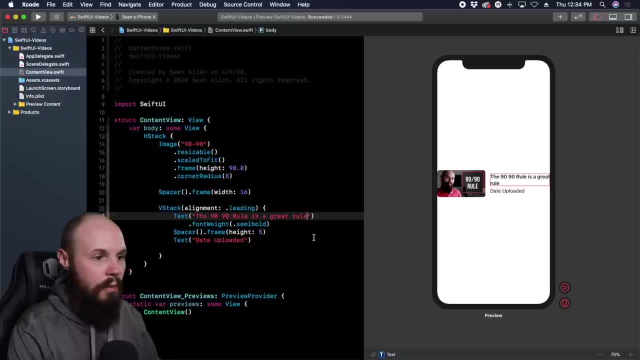 and then we want to limit the lines, because watch if i kept writing. you know, the 90, 90 rule is a great rule. it is so awesome i'm going to misspell this. whatever, it should be three lines. like you can see, our label just keeps growing, and growing, and growing. well, we want to limit this to two, uh, two. 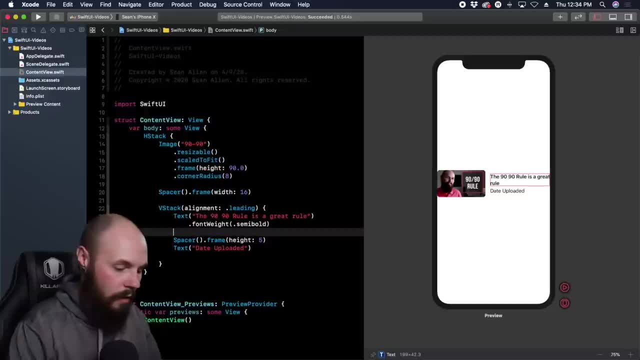 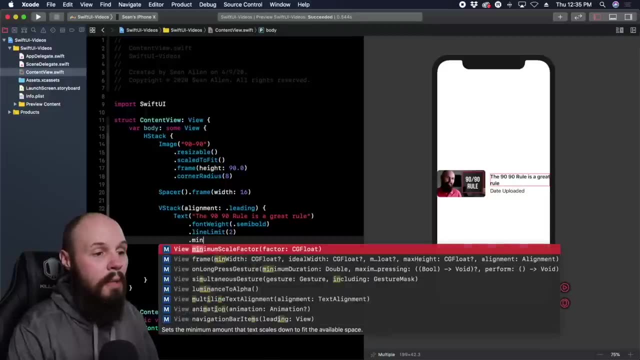 lines because again, you know our title shouldn't be that long. so we can do that. dot line limit makes sense two, so that way it's always going to be. uh, just two lines, and then you can do dot minimum scale factor 0.25. this means like, hey, if you get to that line limit of two and you still 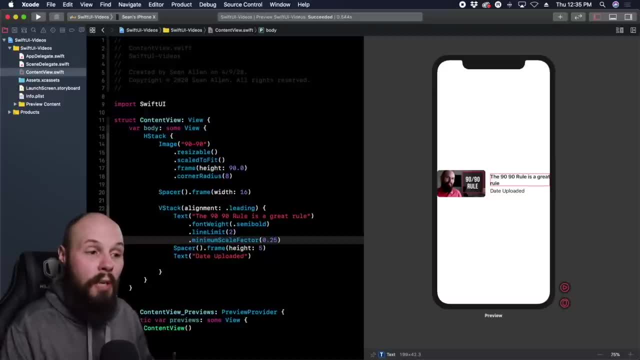 have more words. you can shrink the size of the font and you can do dot minimum scale factor up until 25. that's actually pretty low. we're going to make this like 75. that way it only shrinks a little bit before truncating, rather than making like a size 4 font that you can't even read. 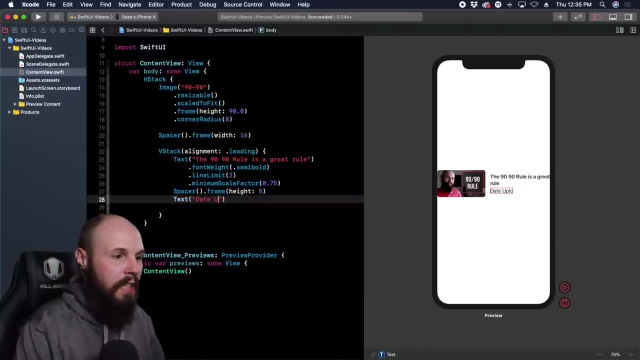 and then similarly onto our date uploaded again. let's just put a sample date in here so we can get to like really see what this looks like. uh, january 23rd 2020. that's not the real date, but we want to see it. so we want to give this a different font, um, or a font type here. so font. 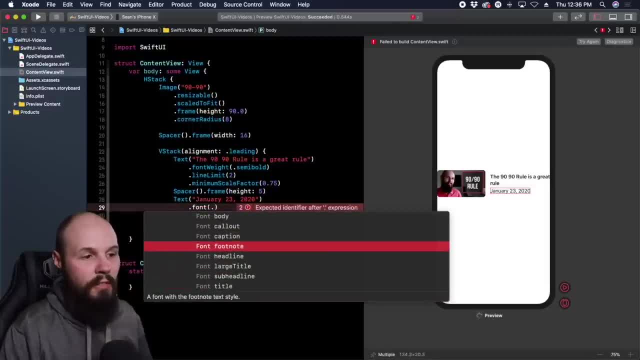 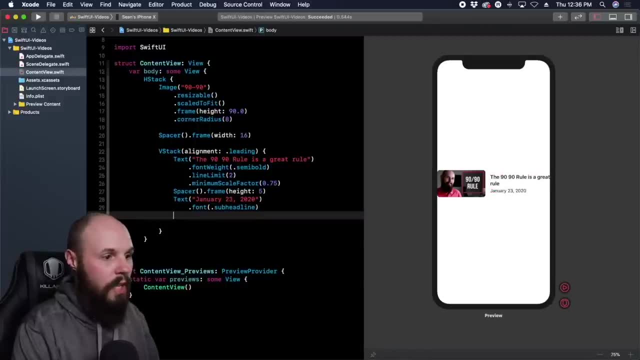 and we want to do dot sub headline. again, you can do different, like follow uh, call out footnotes, caption. large title sub headline makes it a little bit smaller and we can also give it a color. so dot foreground color. and we want to do dot uh secondary. so again these 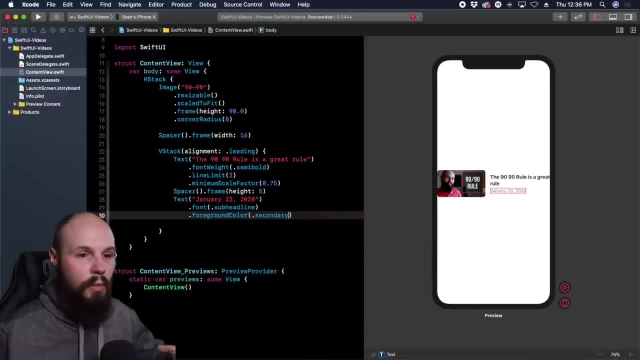 are the um system, ui colors, that'll you know, change via dark mode and light mode, a secondary color. right, it kind of makes sense. the primary color is like the big bold black on a white screen, or it'll be white on a dark screen. the secondary color will be a little bit lighter, as you can see. 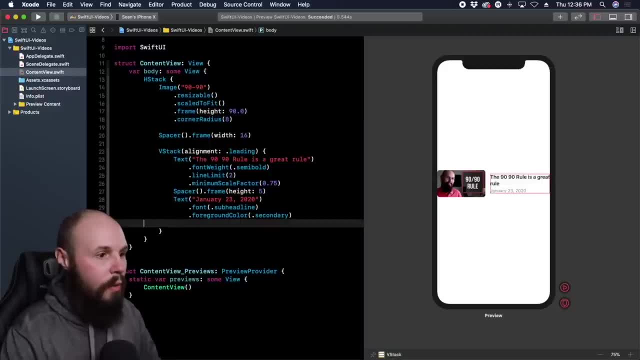 here on our canvas of january 23rd. so that is how we want to format our text. now you may notice we're pinned all the way to the edge on the picture and pinned all the way to the edge on on the text right. there's no padding there. 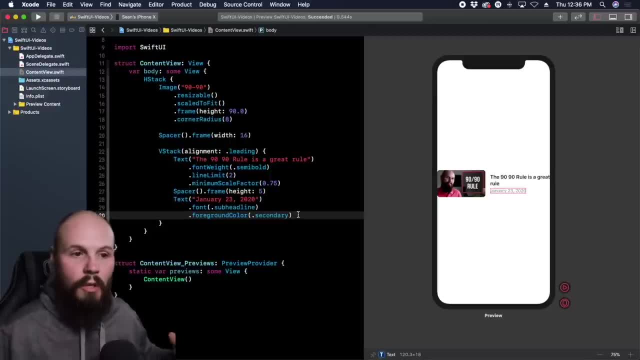 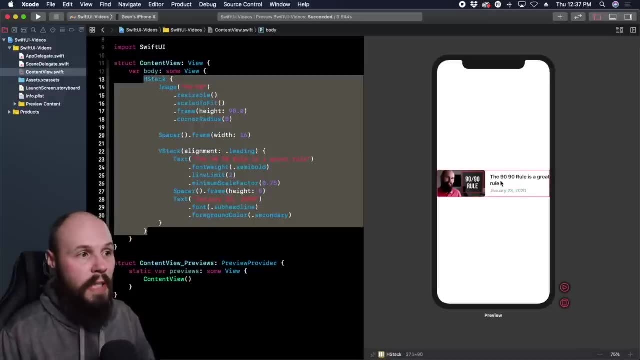 well, when we put this into our list or our table view, that's going to take care of that for us. now watch this right. so here's our h stack. right, our h stack embodies this entire view we just created, right with the image, uh, that we formatted. on the left side of the h stack there's a small 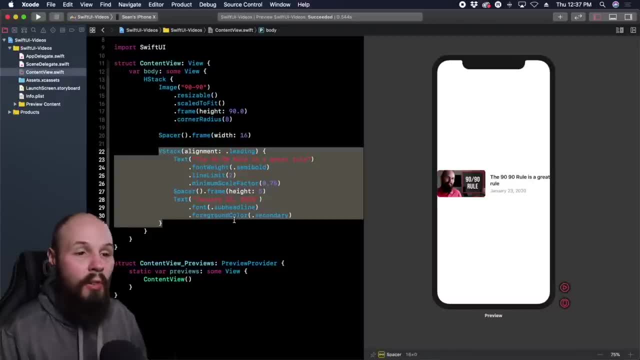 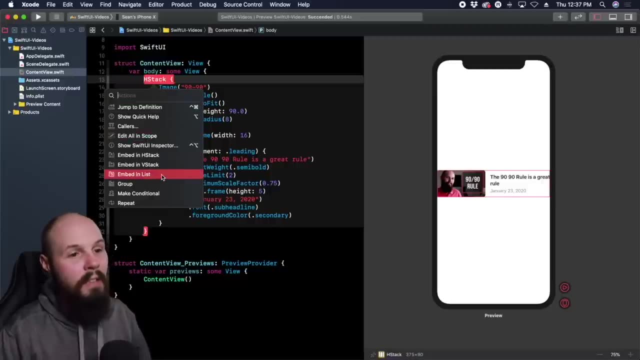 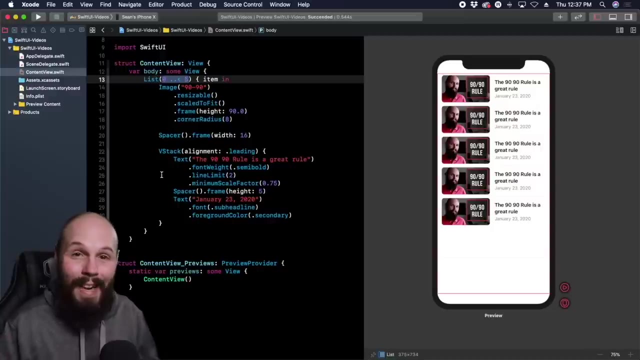 little spacer in the middle to give us that padding. and then we have a v stack on the right of the h stack that holds our text. well, watch, if i do command. click on the h stack. look at this. embed in list, bam, table view. embed in list, you get a table view. of course we gotta format it and change it, but now we have a table. 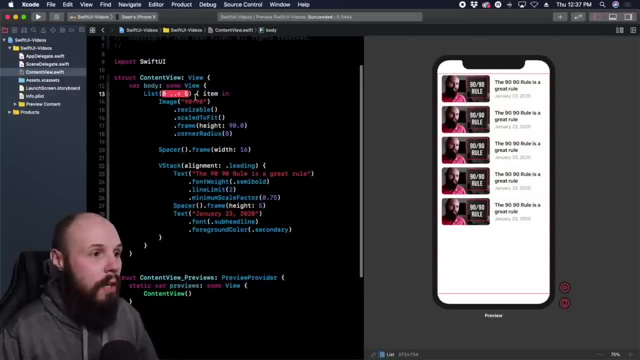 view like that's crazy. and you can see here: uh, the list is zero, uh, up until five. so that's gonna give us five images. but you can imagine if we change that to zero dot dot dot, uh, up until you know 20.. that'll give us 20 of them. as you can see, our canvas filled. and then, if we run it, this: 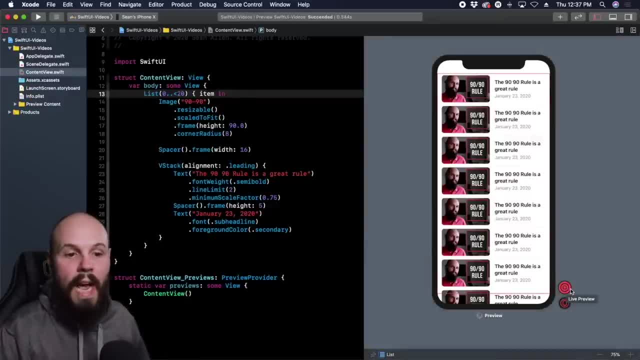 little play button here will run your preview. so hit that and now you're getting essentially a simulator here, once the preview is done, loading uh, that you can actually interact with and use on your app. so here we are. look now scrolling up like that. that was like what? 20, 20 items again. so our basic table view, like we literally just 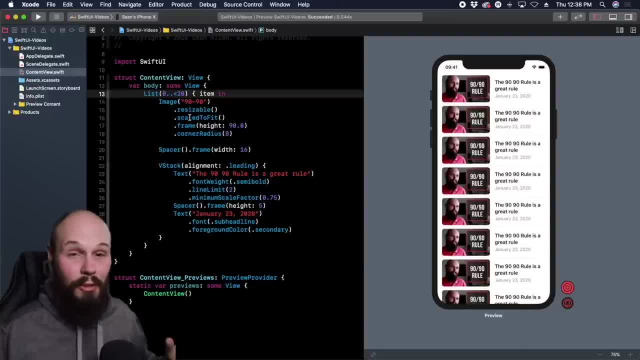 built a view command, clicked it and said, put it in a table view. and it did it like that's crazy. and now, if we're scrolling down here, you notice it's going right up to the top of the screen. um, what if we want like a navigation bar up top? well, that's pretty simple too. now we want to wrap. 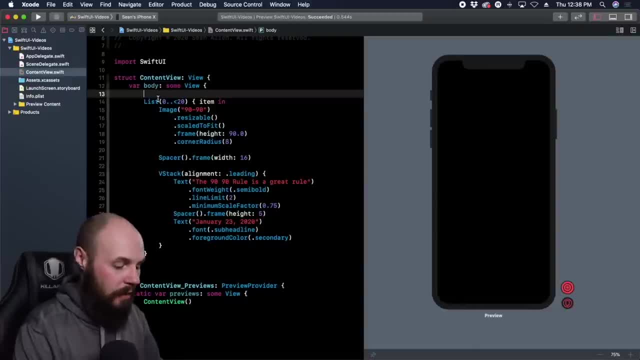 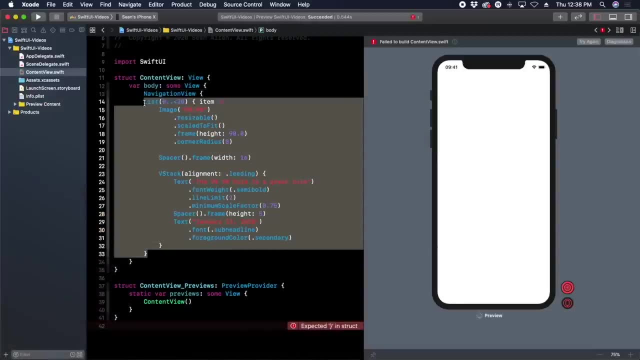 our list inside a navigation view. so we're going to go ahead and do that and we're going to go ahead and do a navigation view. so up here i'm going to type in navigation view. you saw it right there: open and close brackets. um. so this can get tricky sometimes with 50u. i'm not going to lie um like. 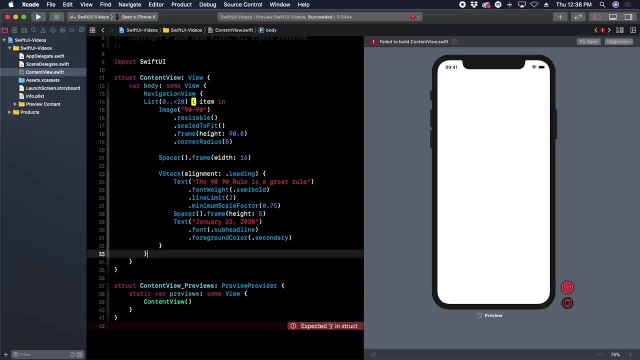 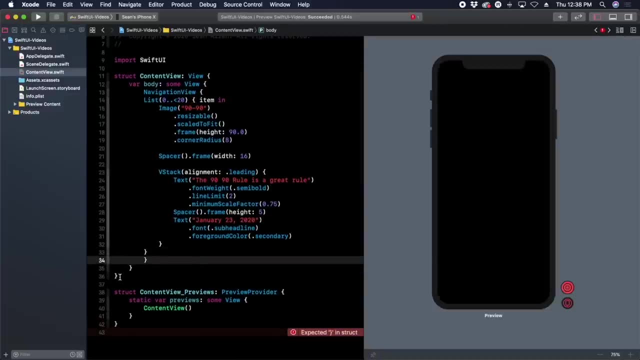 where the brackets go. so if you go left and right over the bracket on your arrow keys, you can see it's highlighting, uh, the list bracket up there in yellow. so i need a bracket below this for the item view. and here's another neat little trick: if you highlight your whole struct, do control, i it like. 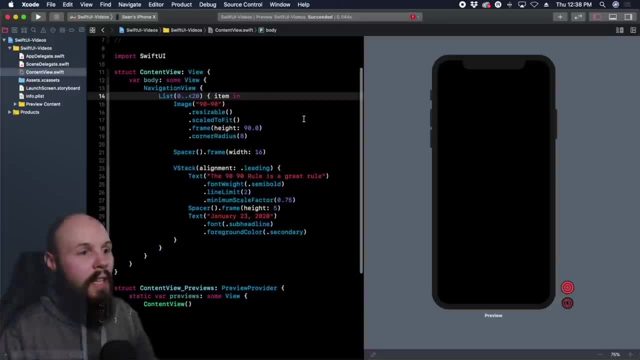 lines up everything for you. uh, the alignment here. so here we have a navigation view. uh, we broke our preview. let's see, here we have a navigation view. uh, we broke our preview. let's see, here we have a navigation bar. let's see, here we have a navigation view. uh, we broke our preview. let's see, here we have. 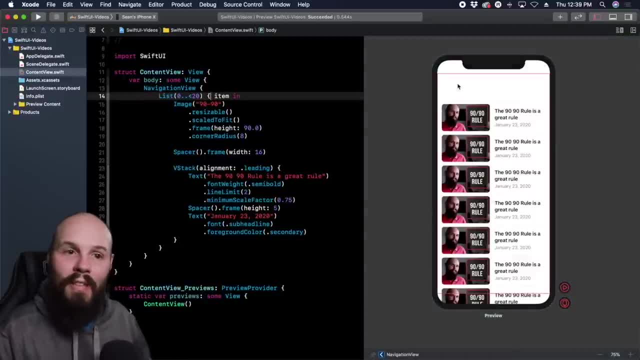 because we like changed the code um, but you can see at the top, now we have like a navigation bar, because we put it in a navigation view and then now on our list we can give a navigation title for what we want this list to be called. so i can do dot: navigation bar title, as you can see here. 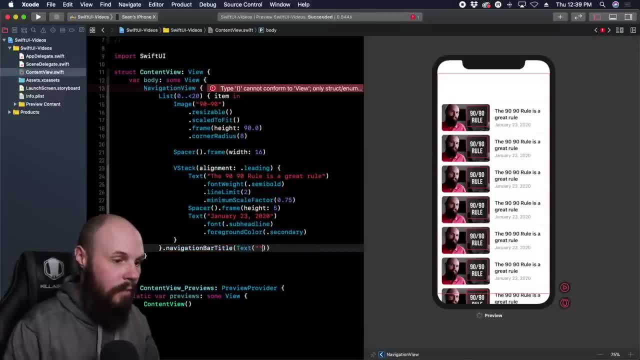 and then we got to pass in a text text of sean's videos and you see it's updating live on our preview. and the tricky thing that you know caught me off guard too is you would think this navigation bar title would be the dot on the navigation. 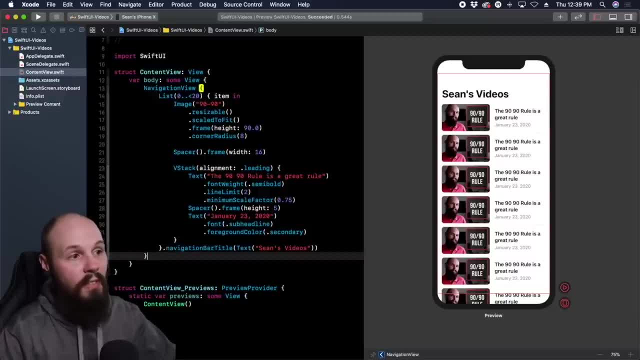 view. right, if i, if i go back and forth on this curly brace, you can see this is the navigation view, curly brace. well, you have to put this navigation bar title on this list here. so little little note in case you mess that up. but now let's run our preview again. 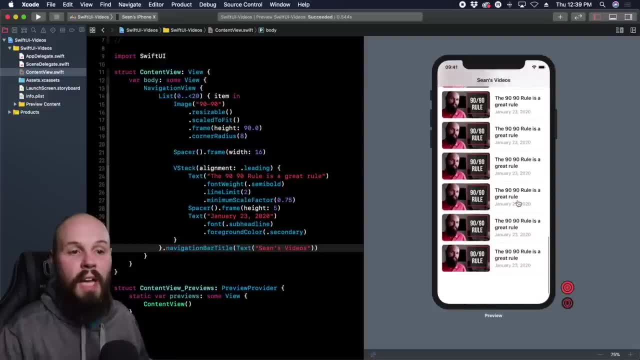 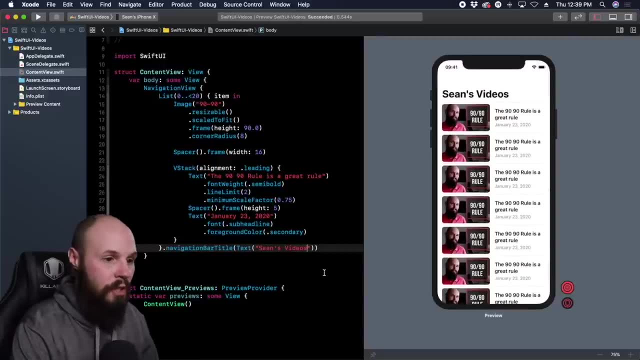 and now look, you see our nav bar at the top. as we're scrolling up, we get sean's videos at the top, just like that, super simple. and look, i'm running my app. right, it's, it's running like on the simulator. let's say i want to change sean's videos to sean's videos, part four. 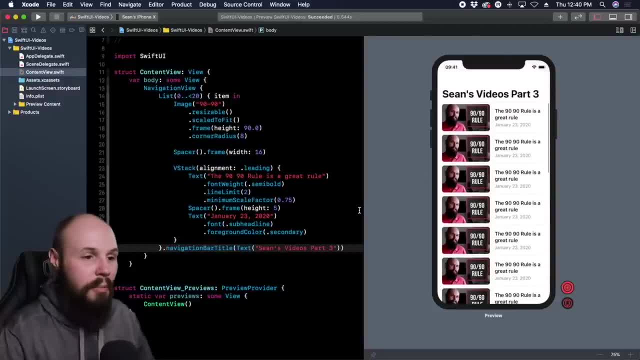 look, it updated right. all right, we're still live. uh, the navigation bar updated part three, not the part four, whatever you get the idea. so, yeah, we're updating this live and it was super quick to create this table view and, you see, when we put this in the table view, it gave us some of the 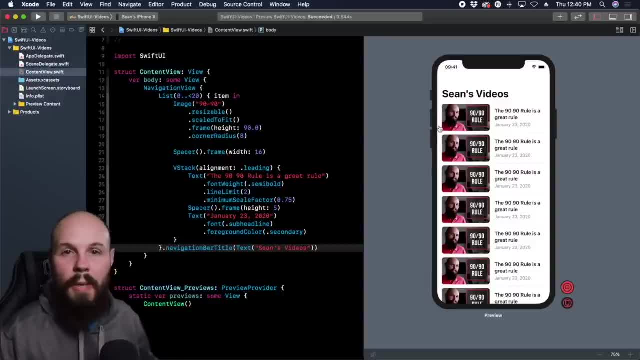 the default padding here on the left. remember before it was in the, the table view. okay, i'm gonna call it table view by accident, but it's really called a list now. um, so that's going to be an old habit to die hard here. but you can see, on the left we get the padding. that's because we 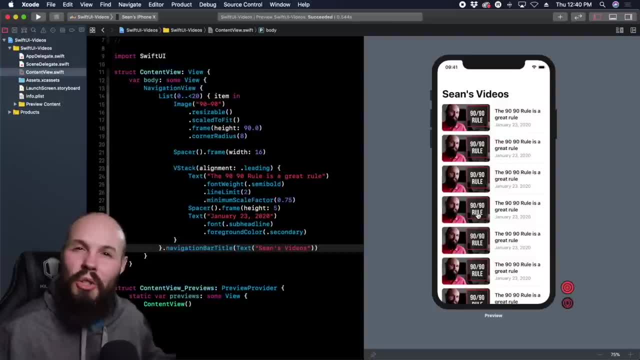 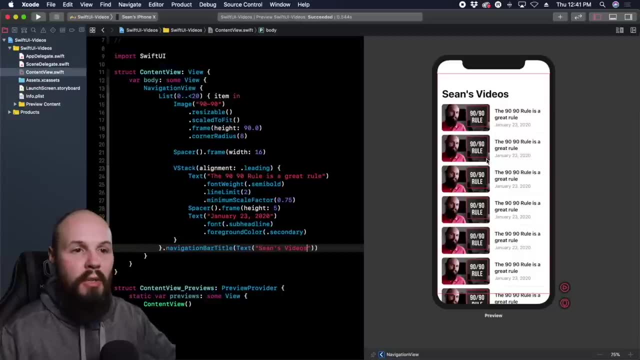 put it into a list and swift ui knows like what a list should look like and it has the built-in padding, built-in margins, like we got everything for free. like that's the power of swift ui. we have our list of videos, but they're all the same video. let's actually put some data in this. 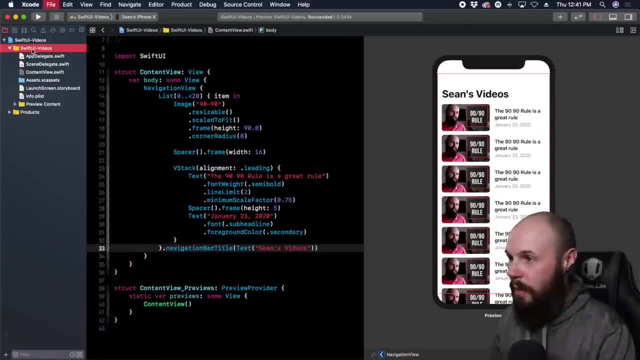 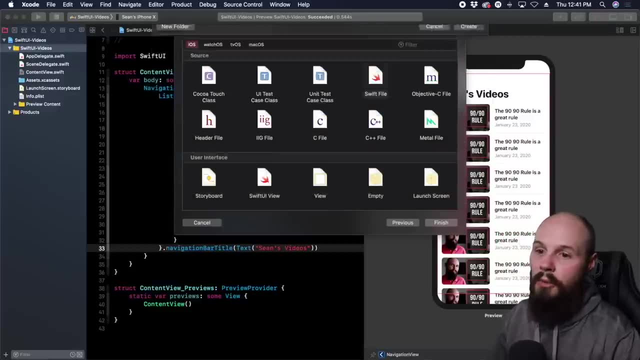 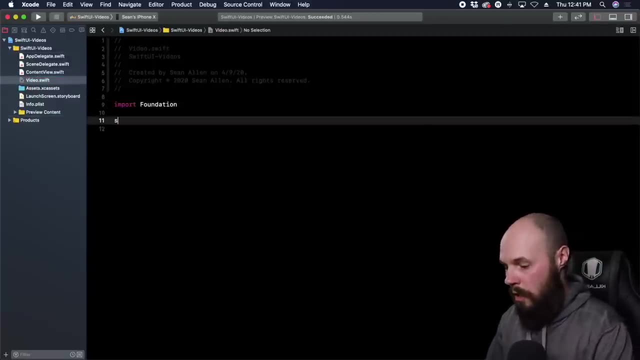 here. so for that, we're going to create a new file in your folder, command n. we're going to create kind of our data model here, swift file. call this, uh, video, hit create. i'm going to drag this up here and here's: we're going to create a struct for our model here. uh, we want to do struct video, we want. 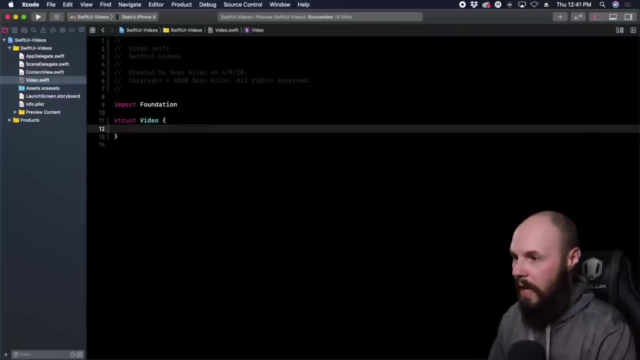 to create a video object here. that video object has three properties, right, it has a var image name- we're just going to get the name of the image, which that is a string. it also has a var uh title. we'll say video, now, just title, that is also a string. and it has a uh upload date, which is also. 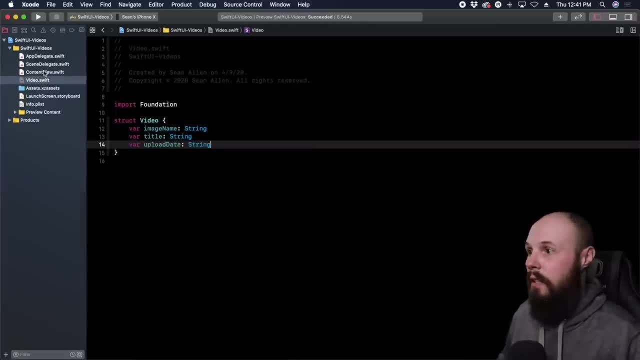 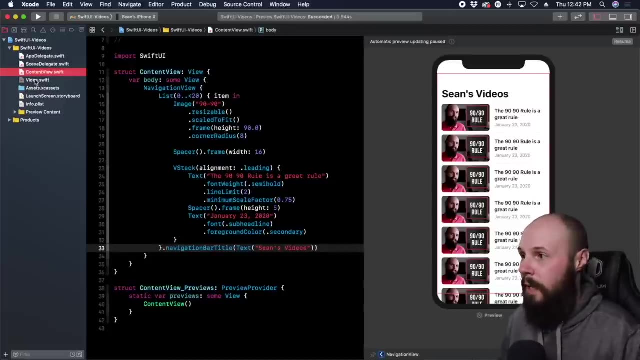 a string that we're going to put in there. so that's our video object. again back to our content view. you can see we're going to have an image name that we're going to create an image out of, we have to pass in a title and we have to pass in an upload date, right? so that's our video now, in order. 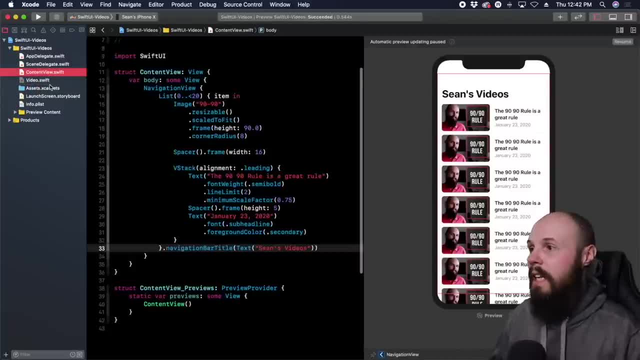 for our list here to use our video object. we're going to create a new image name and we're going to go ahead and call it our video object. we're going to call it our video object. it has to conform to a protocol called identifiable. so identifiable that's how it knows what it is and when you're. 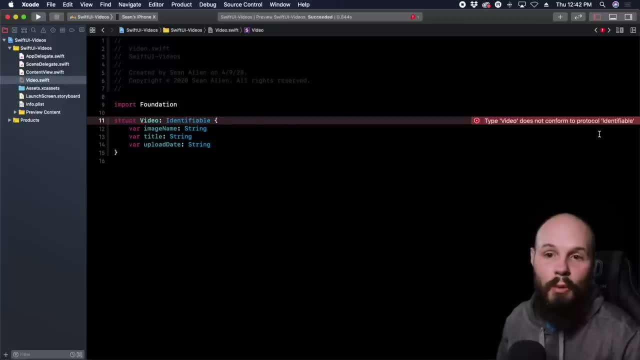 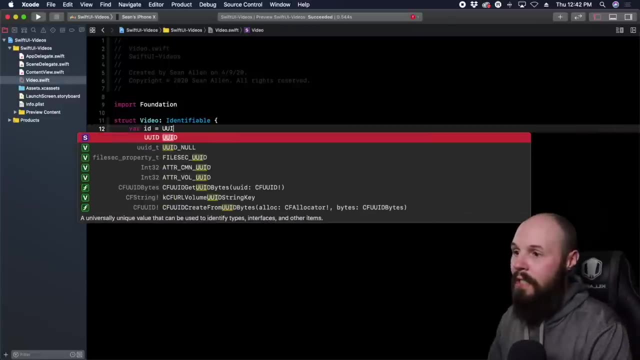 identifiable. you have to have a see. look. it says video does not conform to protocol. identifiable. it's because we have to have a id variable, so do var id, and that equals a uu id and we'll initialize a new one. uu id stands for universally unique identifier, so anytime we create a video, 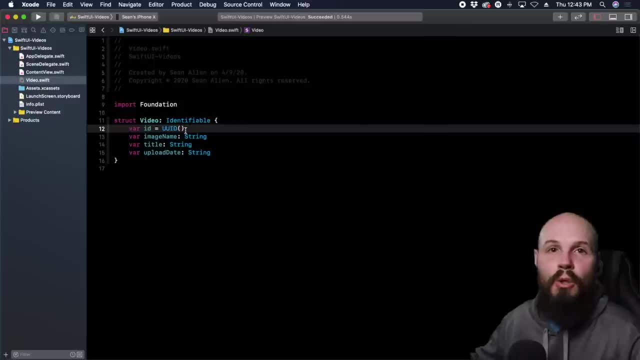 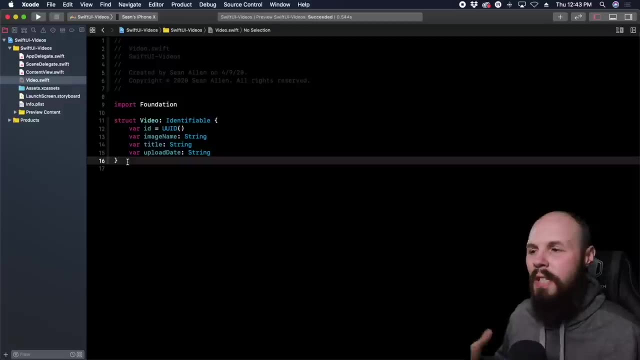 we're. you see, we're initializing a new one, so we're initializing a brand new uu id for this, this specific video object. so we're going to call it, i'm going to paste that in here and then i'm going to. so this is the basic object of a video. now let's create some dummy data, so we'll do that here. 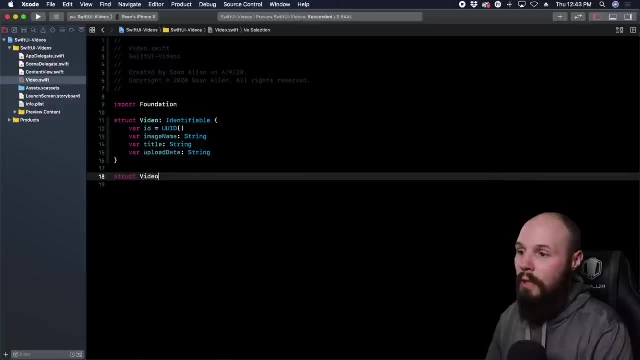 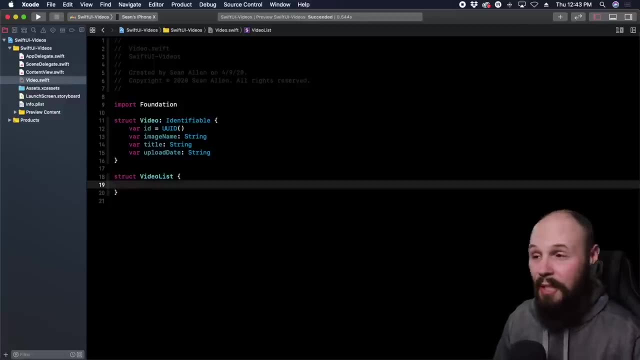 uh, struct video list and this would be the equivalent, like: maybe let's say we're downloading our video list but we're kind of mocking that data here and i'm actually going to copy and paste this because you would watch me type for the next 15 minutes doing this. maybe not 15 minutes. 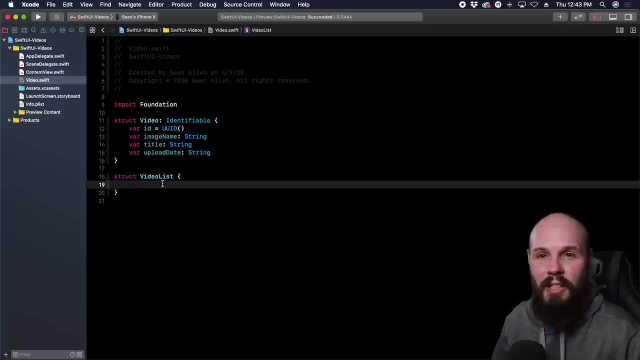 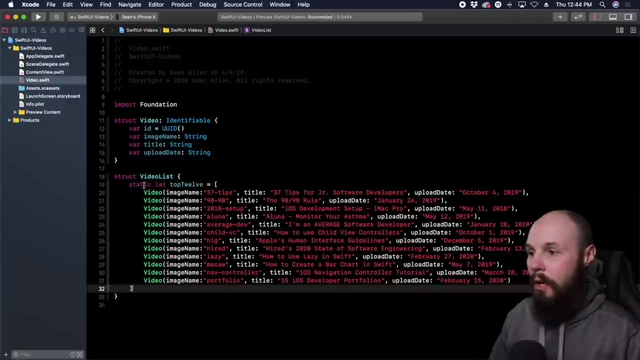 i'm selling my shelf short on my- uh, my typing skills. but let me copy and paste this, and you can pause the video and type it in as well, but i don't want to bore you just watching me type this out. you'll see it's a bit. all right, paste. so there you go. i have a static variable called top 12. 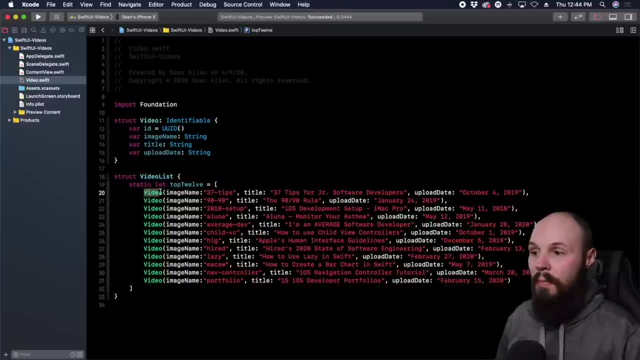 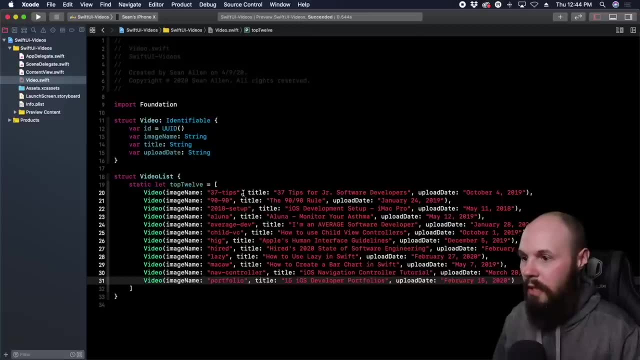 of my video. so this is 12 videos you can see here on line 20, we're initializing a video with an image name: 37 tips. uh, there should actually be a space here. option drag space. there we go. um, it has a title- there's my title- that we're passing in. it has an upload date that we're passing in. 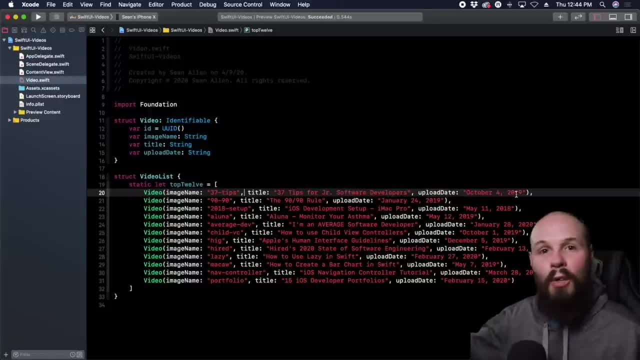 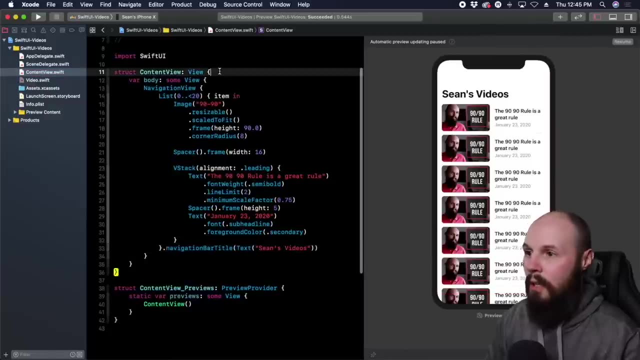 like i said, i manually typed in all this data in a real app. we'd probably be downloading this from the internet, but again, this is our mock data that we're going to use to populate our table view. so back to our content view. we have to update our content view a little bit, so not as part of this uh body. you'll notice this is a. 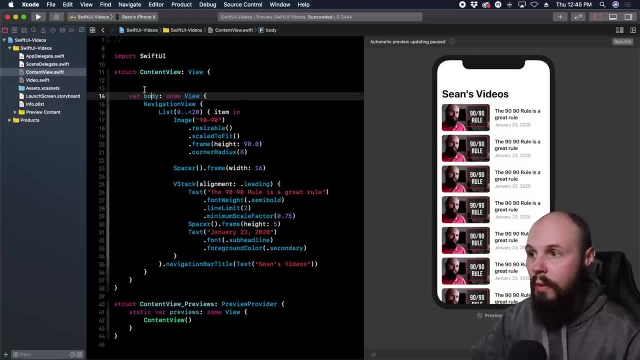 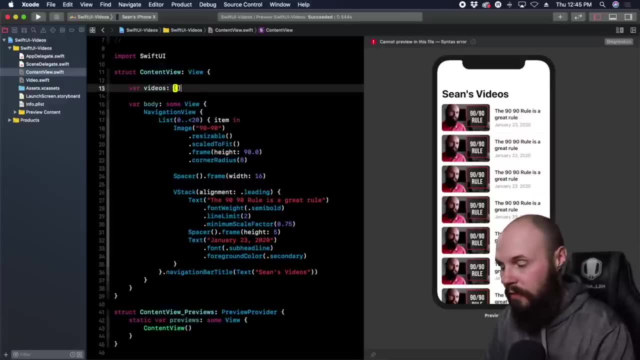 variable called body. that is a view, like our whole screen is like a view, um. so we don't want to mess with that variable, we want to create a new one, so var videos, and you see that is of type an array of video and that is going to equal an empty array right now. so you see, in this down here in the list, 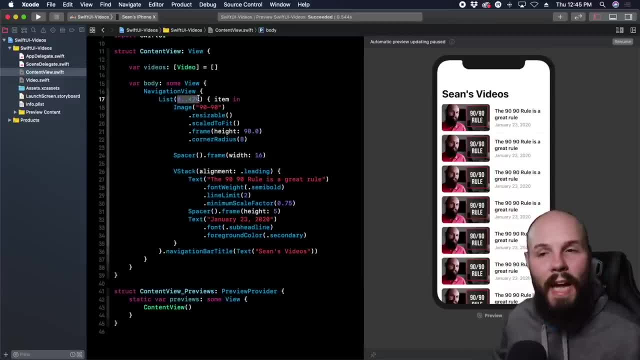 on line 17 instead of 0 through 20. very similar to how um number of rows in section. when we built in uh, a hard coded number, remember we did 50 for the colors app or we could pass in, you know, colors dot count to give it whatever was in the array. it's very similar to what we're doing here by. 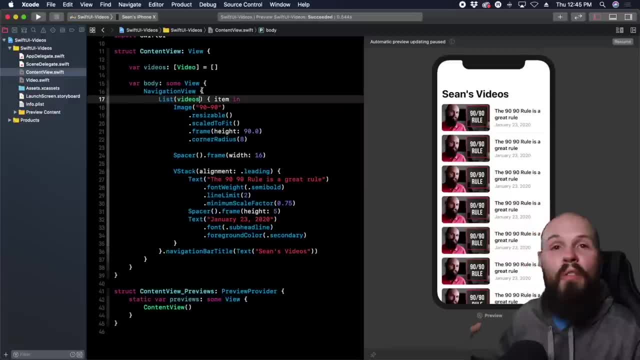 passing in videos. uh, to our list. that is saying however many number of videos are in this array, that is how many cells we should have. and then now item- this is just a renaming item will still work, but that doesn't make as much sense. uh, if we called it video, right, not video, it's just video. 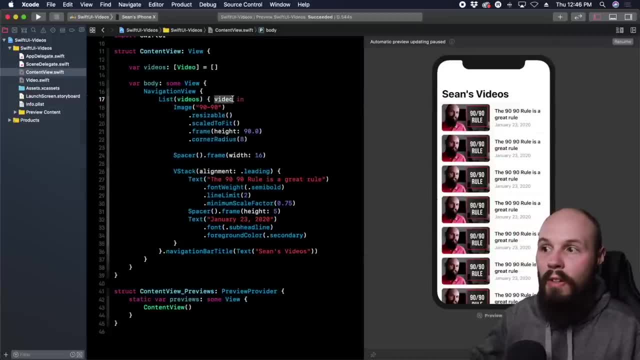 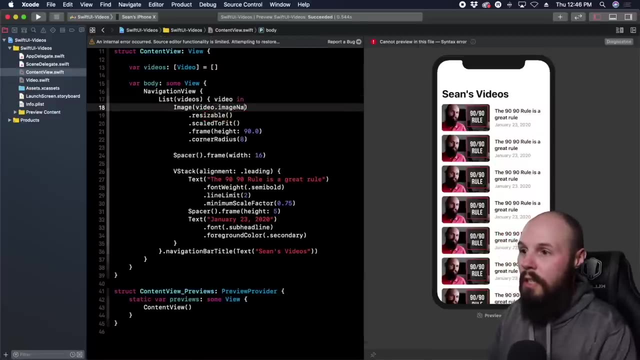 so basically, this is kind of like a for loop right, like for every video in videos. you know, do all that stuff. so instead of the image, instead of passing in 90, 90, we're going to pass in video again. this video is that we have here as it iterates through video dot. image name: there we go. xcode was not. 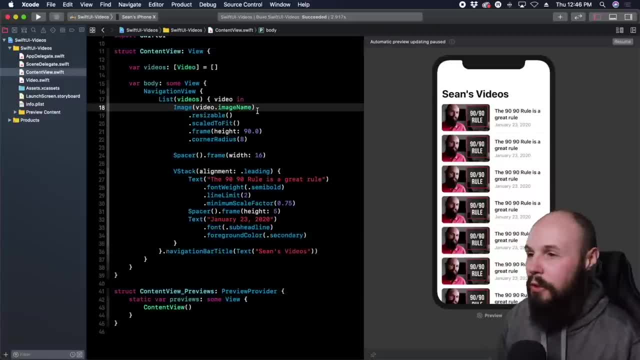 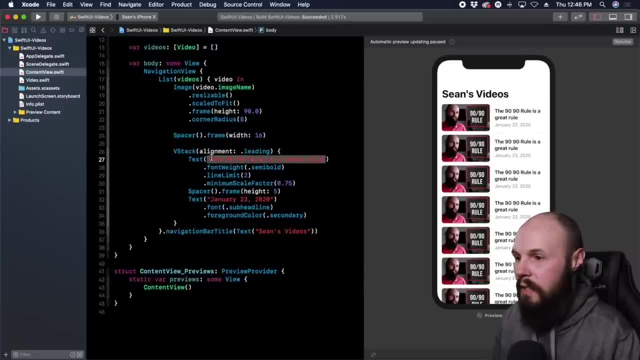 behaving sometimes. that happened especially in swift ui- again super new, um. so video dot image name. same thing down here with the text. we're just replacing the hard coded stuff with whatever video is in the list here. so, uh, we want to do video dot title and same thing down here with the upload date. video dot upload date not getting autocomplete. 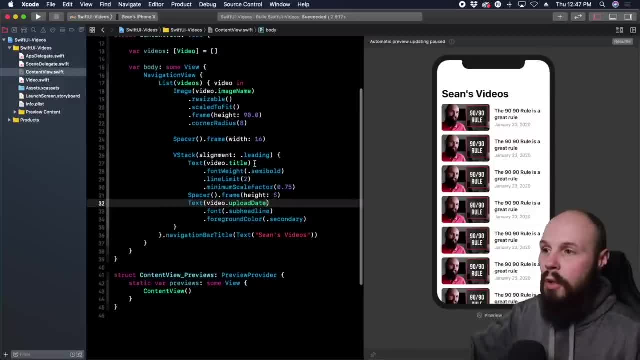 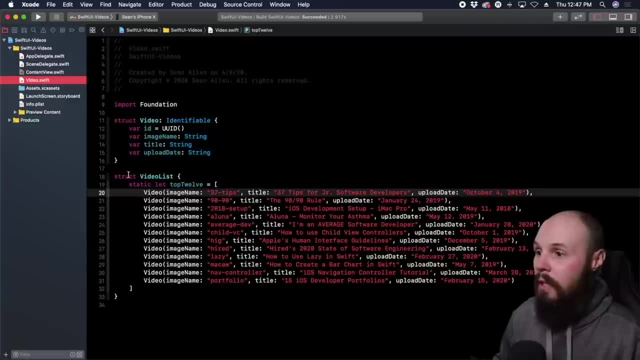 not sure why. um, okay, cool. so we've replaced all of our hard-coded stuff with whatever video we pass in, which again is in this array of videos which we created. again, if you remember, down here on our struct called video list, we created an array called top 12 which has our 12 videos in it. 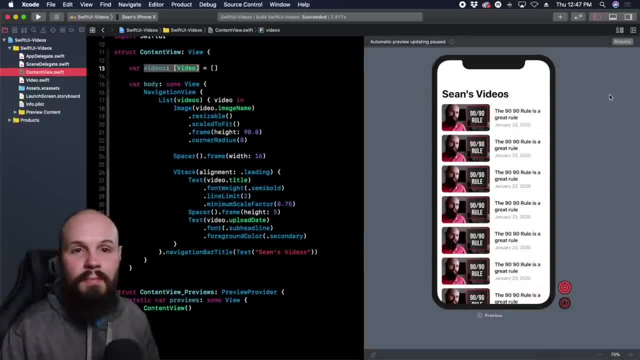 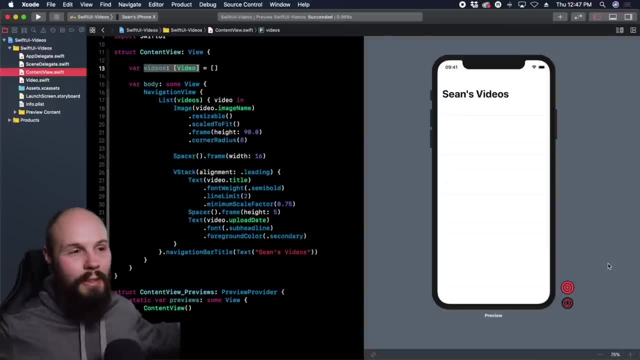 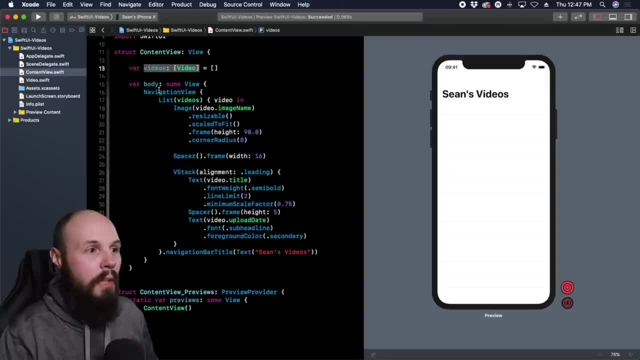 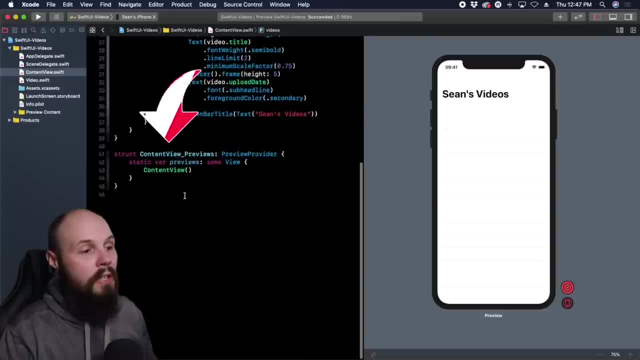 it: um, it's a blank table view because, like, yeah, we changed all this stuff, we haven't, uh, told this array of videos what's in it? right, like it's an empty array. so here in this preview, uh, struct. this is what actually generates the preview here on the on the right: uh, you'll notice content view. 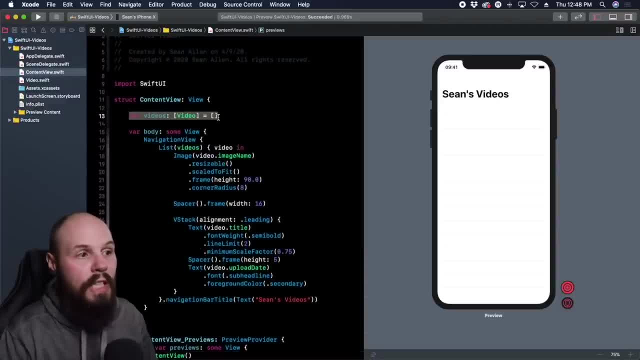 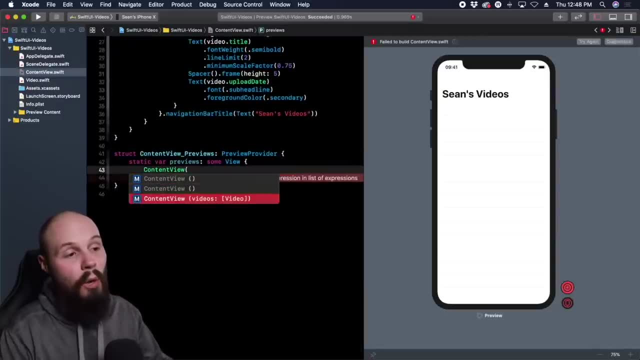 will now be able to take in a parameter, right, because we have a variable called videos on our content view. so watch, if i just delete the initializer there, open it up and we'll see. now we get a parameter called videos that we can pass in. so what this is saying is: hey, show my 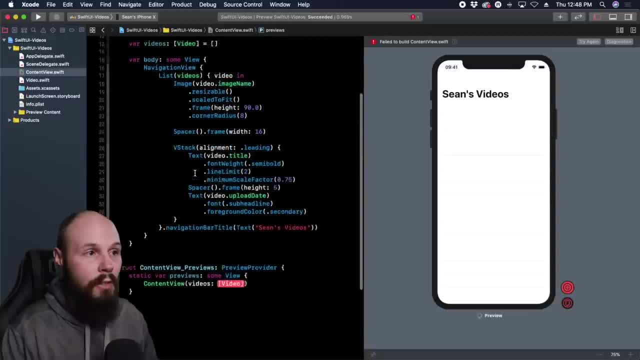 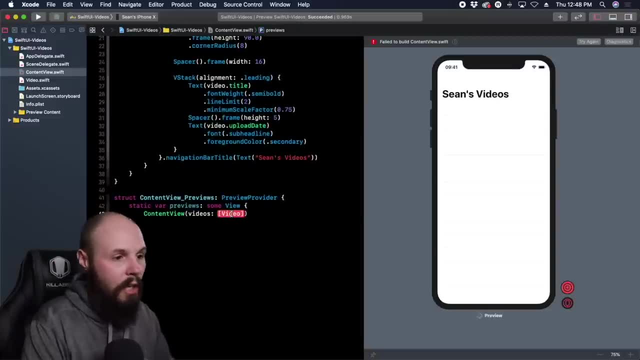 preview but pass in an array of videos to my content view. and again, content view is just this whole thing we've been working on. so what array do we want to pass into our content view? we want to give our content view video list dot top 12, right again, just to reiterate. and you see, look. 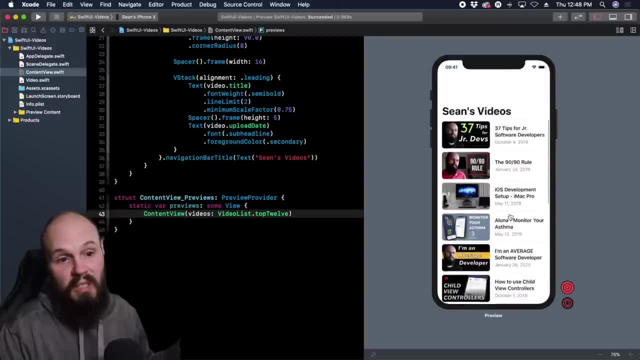 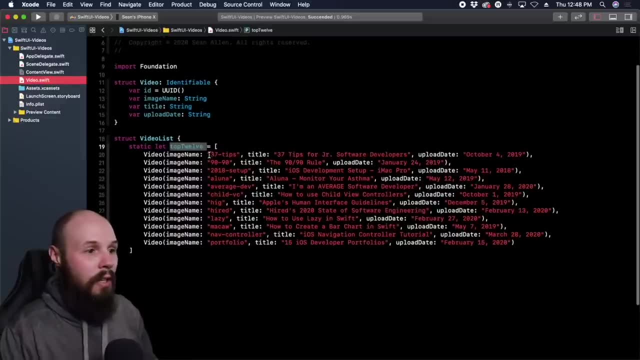 at that immediately updated, bam, and it's running like i can scroll and everything. so you see the power of swift ui and how fast things load. and you see, based on the array of videos that we've created here, you know, with the, the image name, the title, upload date on all those videos, that is. 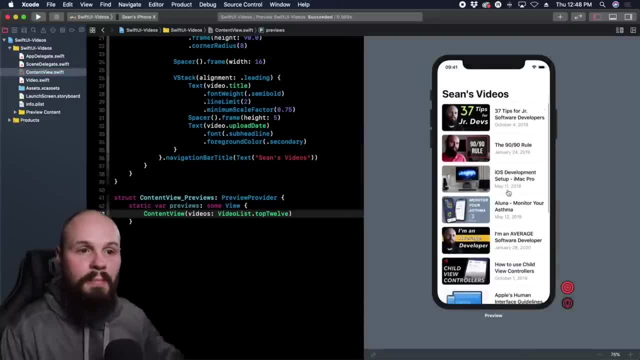 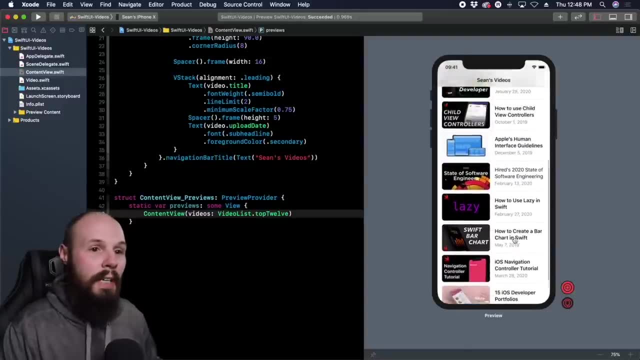 populating here. see, we get 37 tips for junior software developers and you can scroll down through. you know some of my, my recent videos here you see, we get the video image, we get the title, we get the upload date. uh, again, so you saw. yeah, it took a little bit of time because i was explaining. 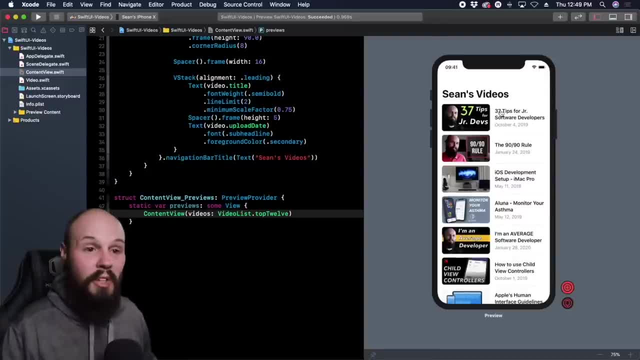 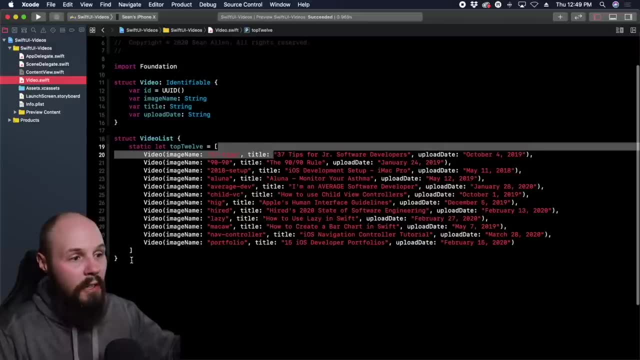 everything and going slow. but we just built this table view with a custom cell very quickly and then again look like here's all the code, like of course we had our data model over here, but like that's a little bit of code, of course, but the ui code. 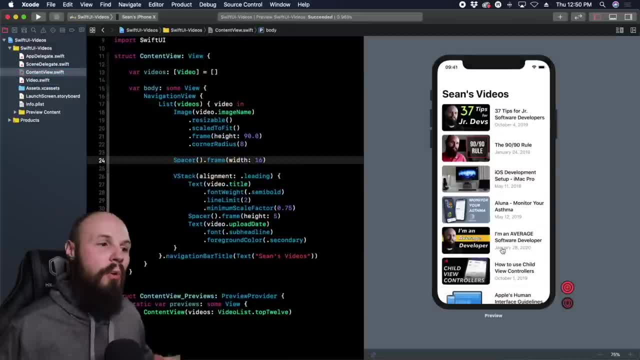 not a lot. so there you have a quick swift ui preview again. you can see it's vastly different. it's a fundamentally different way to program your ui than what we're used to with ui kit. but that was a preview. um, i would say happy to answer any questions in the comments, but to be honest, 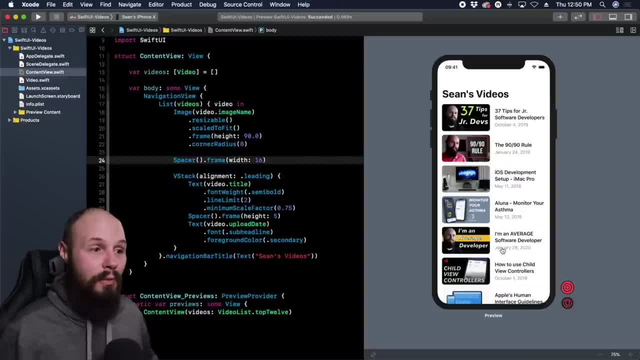 with you. i've only done the very, very basic layer of swift ui, so if you have very deep questions, feel free to ask them and hit up the slack as well. i'm just not going to promise i'm going to answer them. however, like i said, i'm going to answer them and i'm going to answer them in the next video. 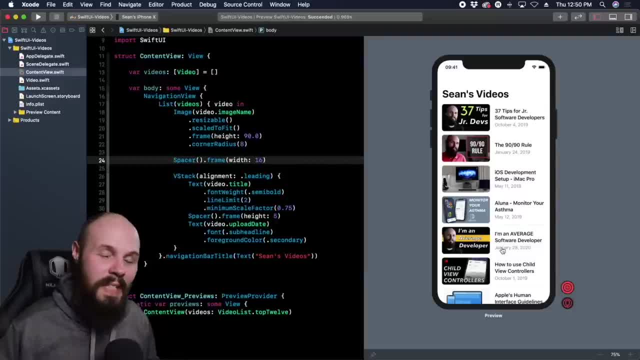 my, my whole year, after this course is released, as of april, is dedicated to swift ui, because i have a product in mind that i'm going to build fully in swift ui and catalyst and have it be across all platforms. so, yeah, so the next eight months, 100 swift ui for me and then, like i said, by the 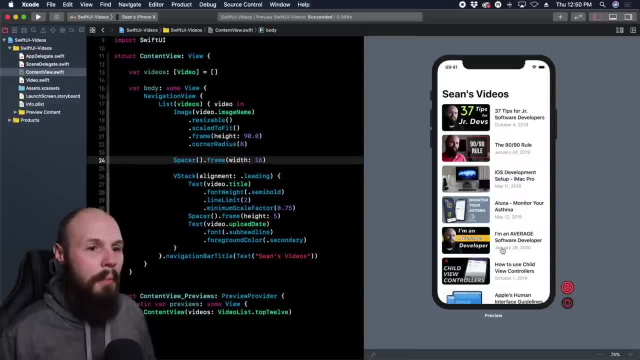 end of the year i'll have a pretty basic beginner course on swift ui, but anyway, that's it. i'm pretty excited for the future of ios development, which is clear that's going to be swift ui again. we're just not there yet and even if you're super excited about this, i i would definitely learn. 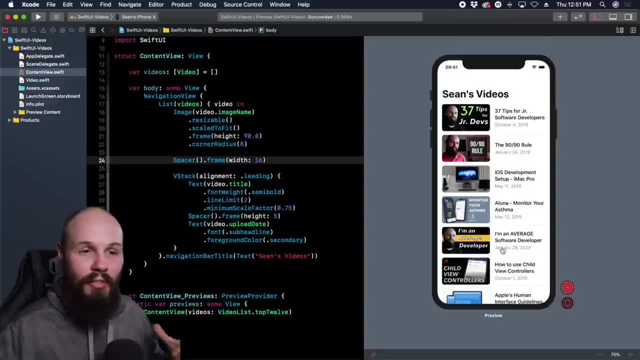 ui and i would definitely learn ui, and i would definitely learn ui and i would definitely learn ui kit. first and again, like i said, swift ui is going to go through a phase over the next year or two of constant changes and we're figuring it out, but anyway, that's the preview. hope you. 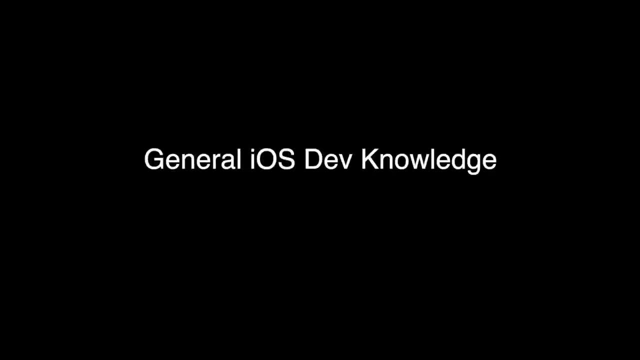 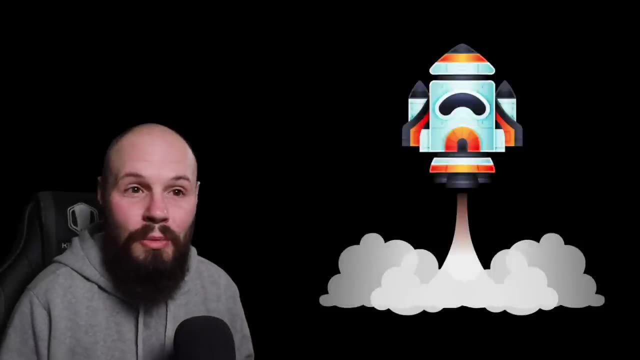 enjoyed it on to the next video. so many times when i was just learning, i remember hearing about a concept and being like i didn't even know that was a thing, like i didn't know that existed. well, that is what this section is meant to help out with. as i've said many times, the goal of this course is to expose you to this world. 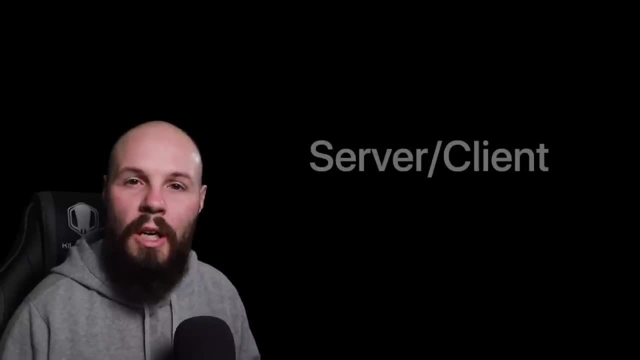 so i don't want you to be overwhelmed by these topics. we're going to talk about how most apps typically work, you know, between a server and a client right. for example, if you're on twitter, your tweets got to live somewhere and that's off on the server. we're going to explain how that. 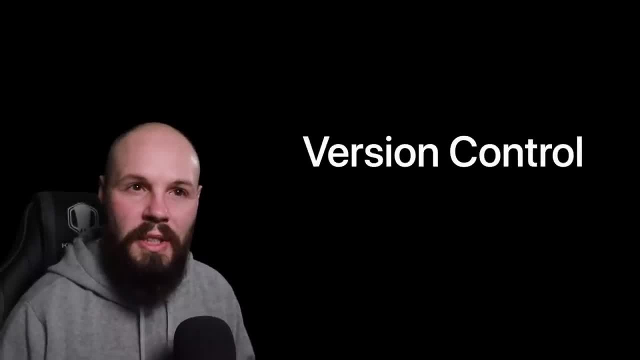 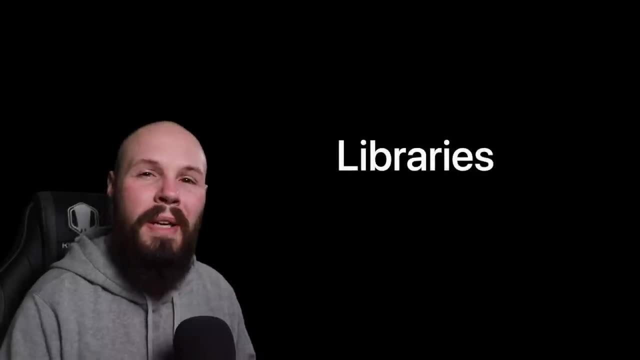 process works. we're going to talk about version control, which is essentially, you know, a save state for your code base and it allows development teams to work together. we're also going to talk about third-party libraries, how you can bring in, like a module of other people's code into your program. 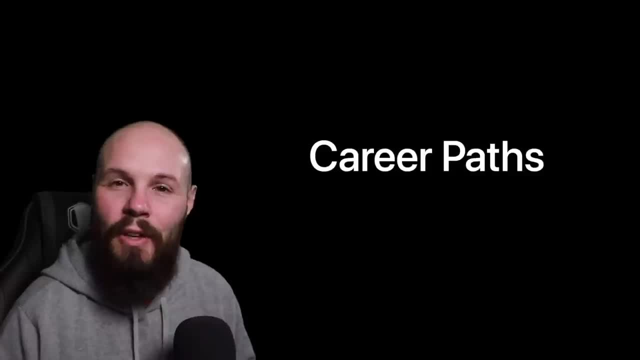 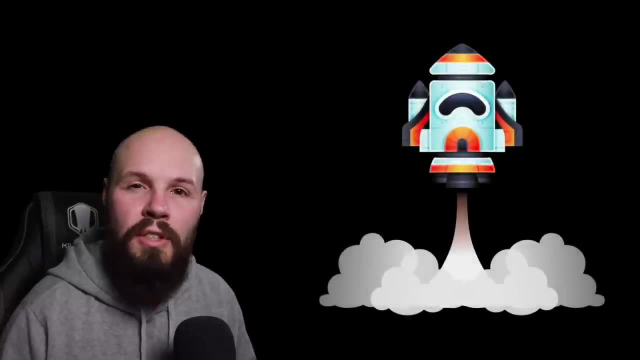 and then we're also going to talk about various career programs and we're going to talk about different ways that you can take a career path. a developer can take right, you can go big company, you can be a freelancer. we're going to dive into that now. as i've said before, the whole goal of 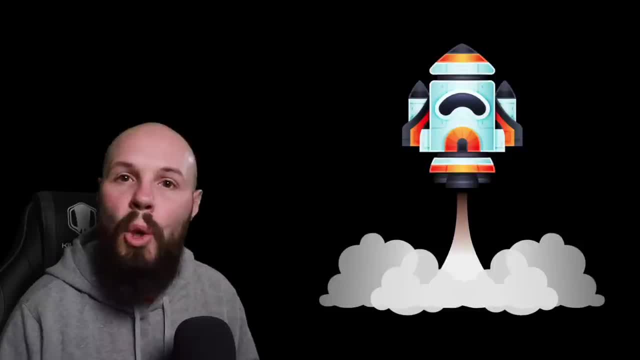 this course is to just expose you to this world, so please don't feel overwhelmed when you're watching these videos that you don't know this stuff, the concepts in these videos could be entire courses in and of themselves and again, i don't want to overwhelm you but, like i said, i want to let you. 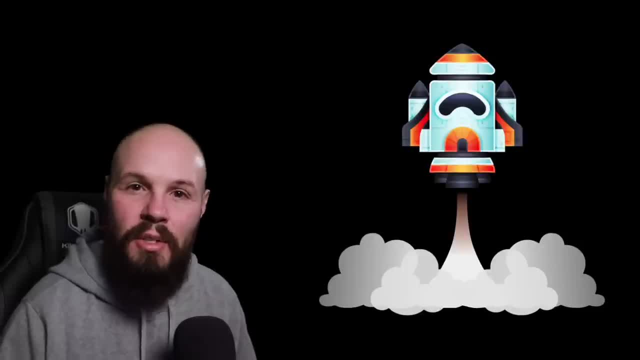 know that this exists, so don't worry if you don't fully get all these concepts yet. these are things that you will learn journey. they're not really for absolute beginners but again, like i said so many times, i was like i didn't even know this existed. well, again in this section, we're trying to fix that problem. 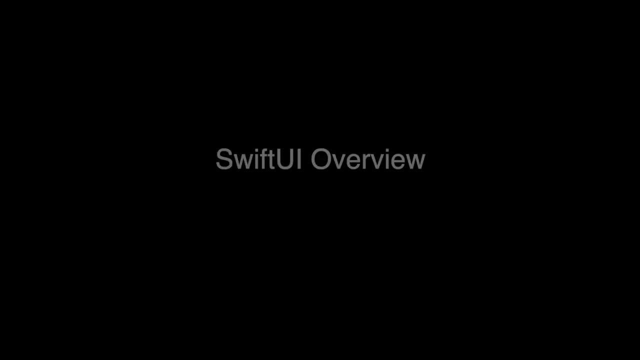 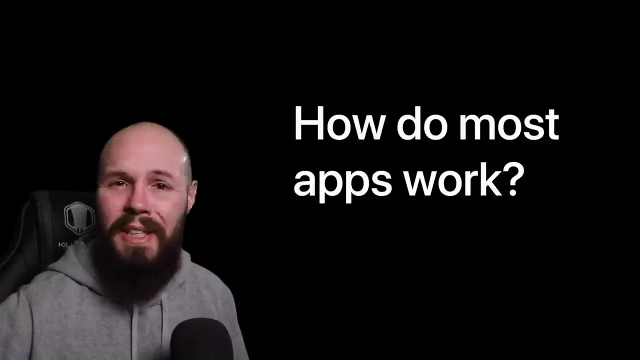 so how do most apps work? obviously that's it's a pretty broad question and could be 20 courses in and of itself to explain everything. so, of course, we're going to keep this high level simple and we're going to talk about apps that deal with the server and client dynamic, which again is 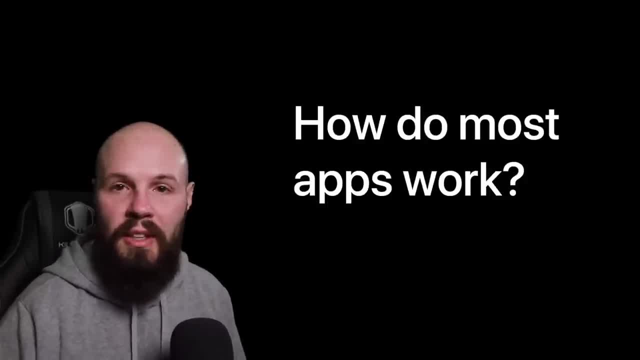 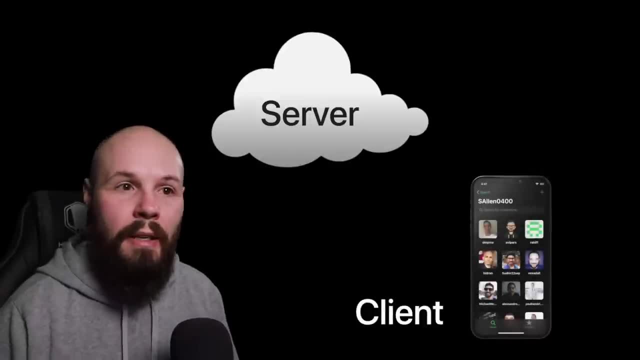 the most apps. first, let's simply define, you know, server in the client. so the server is something you may think of as like the cloud and the client is either your phone, your ipad, maybe your imac, your, your laptop, like that is the client. so, for example, let's take twitter: right your tweets, they live in. 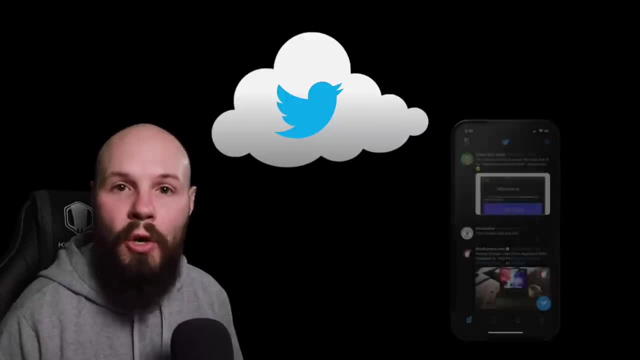 twitter servers right, they live off in the cloud. however, when you open up your phone and pull up twitter, the server sends all those tweets and all that information to your phone. the client, and then the client you know, processes that information and displays it to the client and then the client. 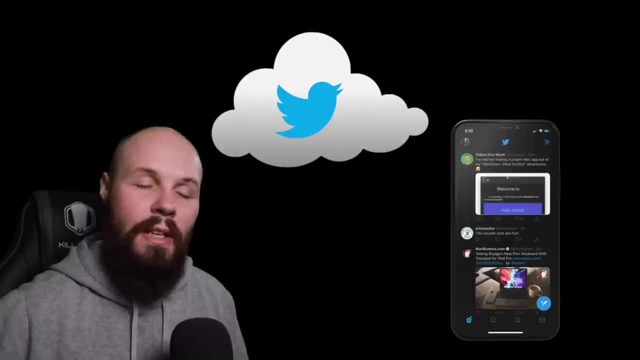 displays it on the phone. so again, all the data lives on the server, right, all the tweets, all that stuff. and then you have to have wi-fi or a cellular connection to pull that down from the server. so why i reiterated that? is because i want to talk about that data that gets passed. typically it's via json. 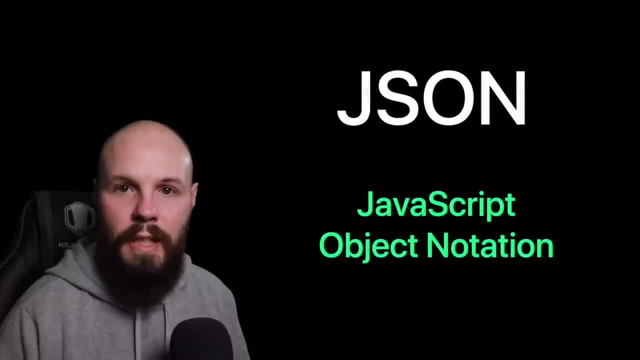 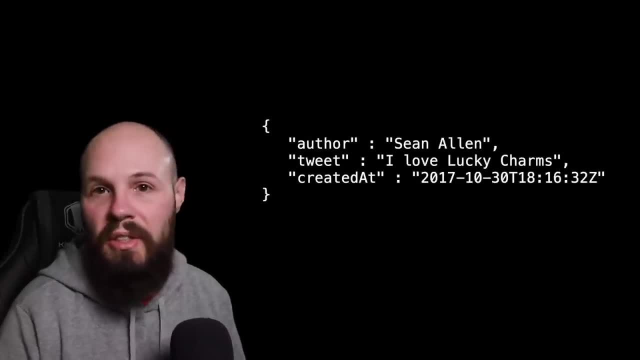 json or javascript object notation. here on the screen you can see a very simplified json of what a tweet might be right, you can see who tweeted it, you can see the tweet message, you can see when they tweeted it. and i say this is an overly simplified version of the tweet message. but 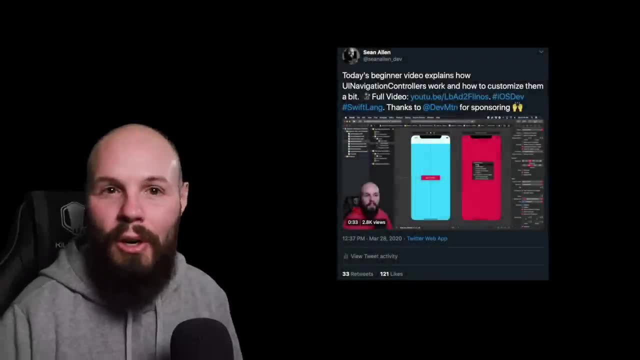 you can see that the tweet is a very simplified version of a tweet, because the tweet is going to have a lot more data. right, you have like the avatar. if the tweet has a video or an image, you got all the people that liked it, all the people that retweeted it. so, again, this is just a super 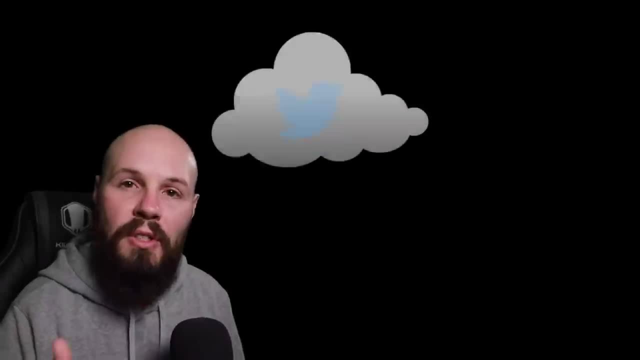 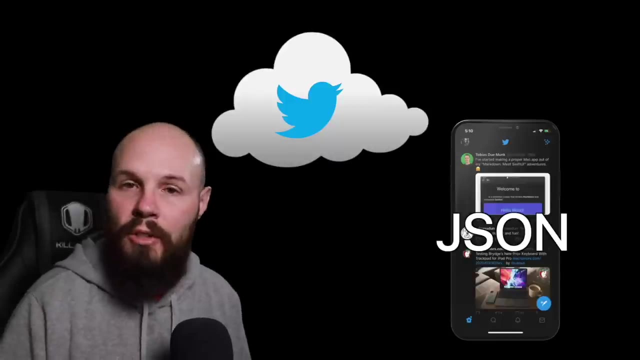 simplified version to illustrate the point. so what gets sent from the server, again the cloud, to your phone or your ipad or your computer is a list of these json objects, that are the tweets. so the client's job, which is again the phone, the ipad, the computer, is to take this json parse. 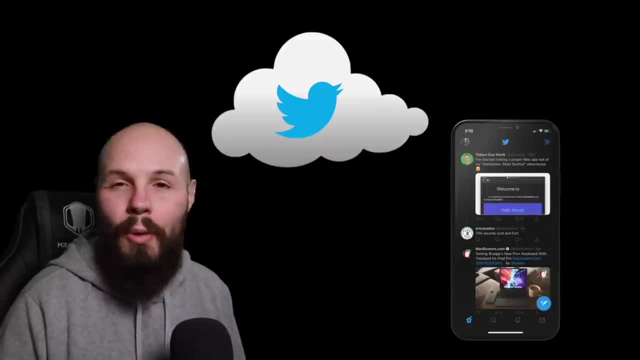 through it and make it look pretty on the screen. so the client's job is to take this json, parse through it and make it look pretty on the screen, right like the running joke is that 90 of ios development is just hitting a server parsing the json, making it look pretty on the screen. and it's not far from the truth. like this is a core. 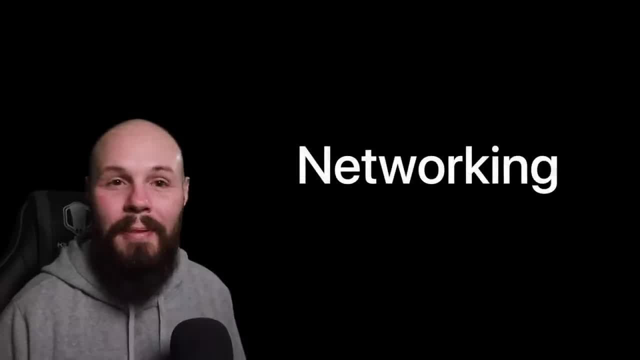 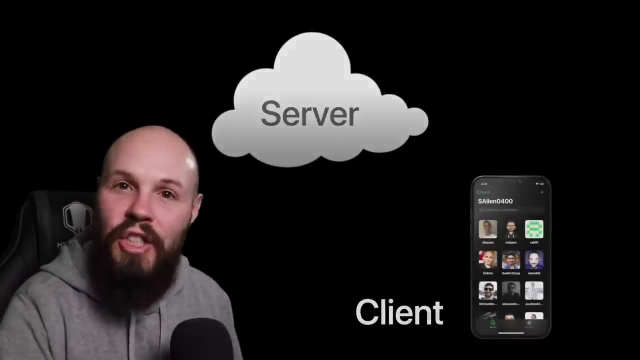 fundamental skill in ios development. this is called networking. however, networking isn't something super beginner developers need to learn, even though it's a fundamental skill. it's something you're going to learn later on in your journey. but again, just knowing the fundamentals of of the server, the client, seeing this json that you know that you have to parse to. 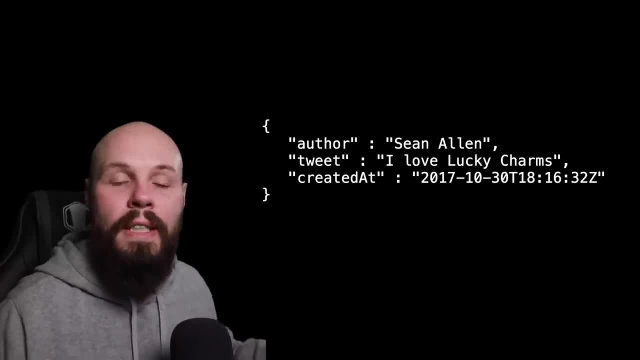 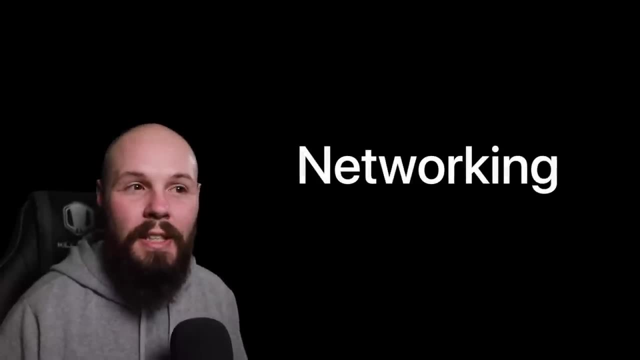 make look pretty on the screen. just knowing that at a high level gives you a head start when it comes time to learn networking, because ask any developer that's gone through this journey. networking is one of the more difficult things to learn and it always trips people up especially. 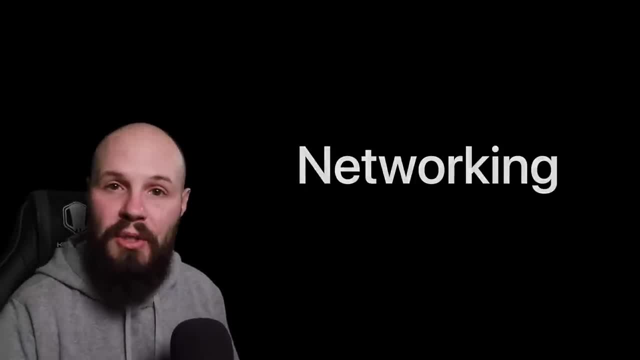 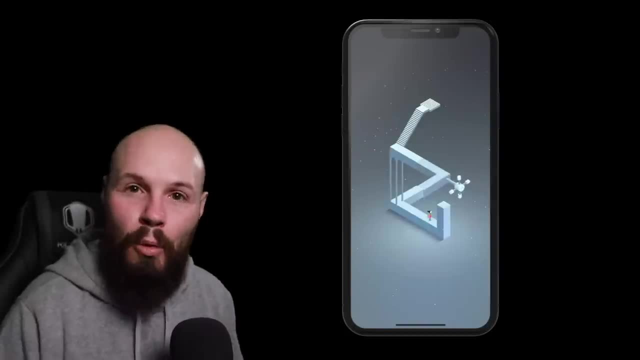 parsing through the json now again. not all apps have this server client dynamic. like some apps, typically games, uh. all live on your phone. so if you ever had an app or if you deleted the app, you lost all the information on the app. that means no data was living on a. 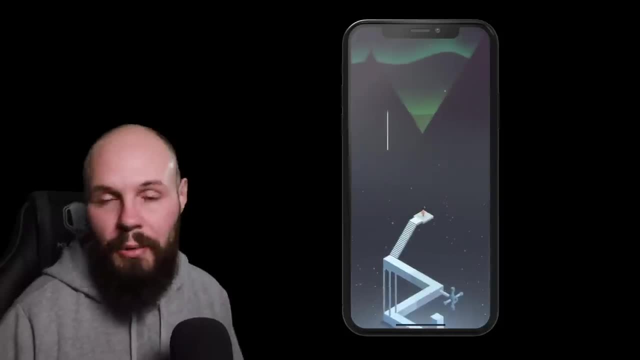 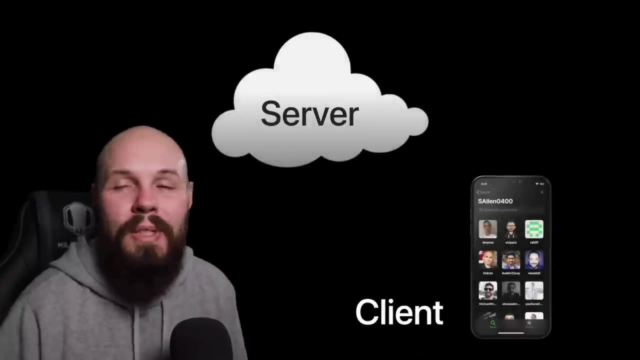 server, all the data was living on the client, which is the phone, the ipad, the computer, uh, so that's a different dynamic. um, but again, most apps- the, the facebooks, the instagrams, the twitters, like most apps, have data on a server right, because, in this day and age, you want to be able to log. 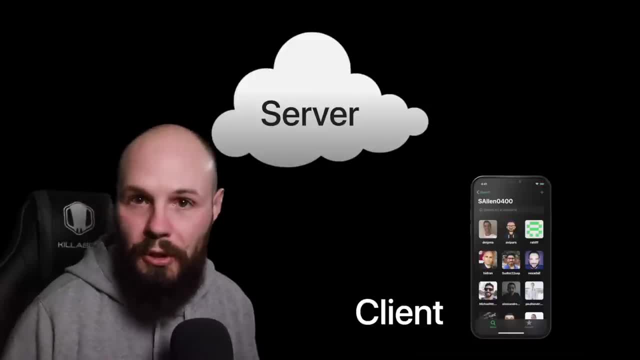 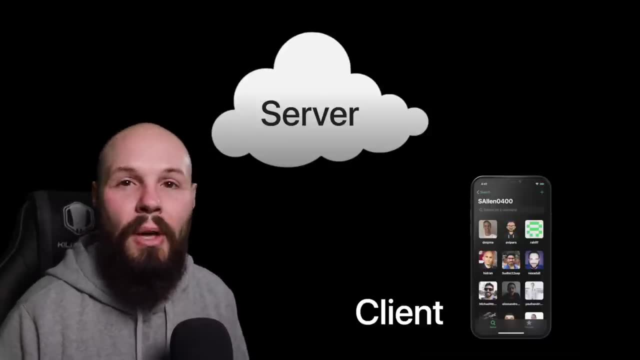 onto your ipad and get your the same data that you can log onto your computer and get right. a lot of stuff lives in the cloud, so to speak. so again, this server client dynamic again is fundamental knowledge and we just- i oversimplified this just to be clear. 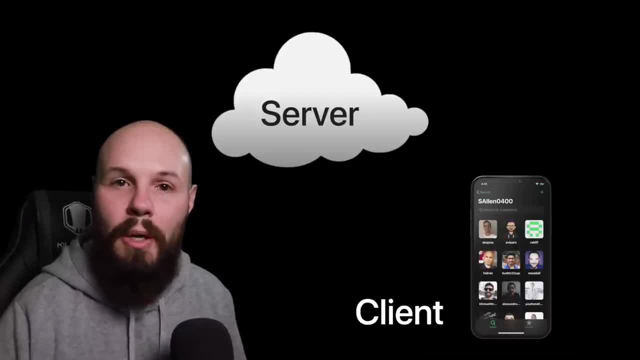 because, again, this course is about just exposing you to this and teaching you just the very fundamentals. so when it comes time to learn this networking, like you, you have the fundamental knowledge of how it all works. now you just need to learn the implementation details. all right, as always, if you have questions, hit me up in the comments or in slack. see you in the next. 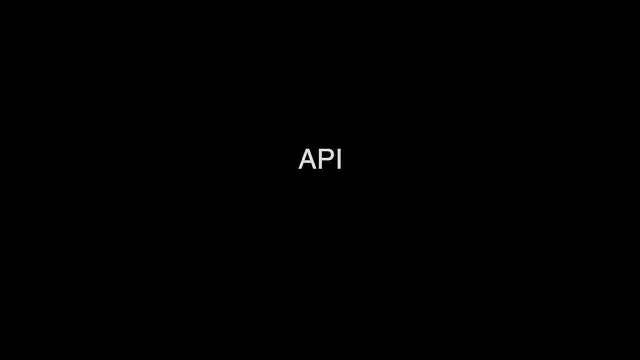 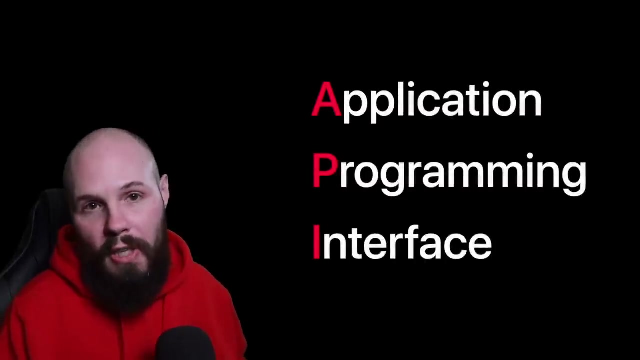 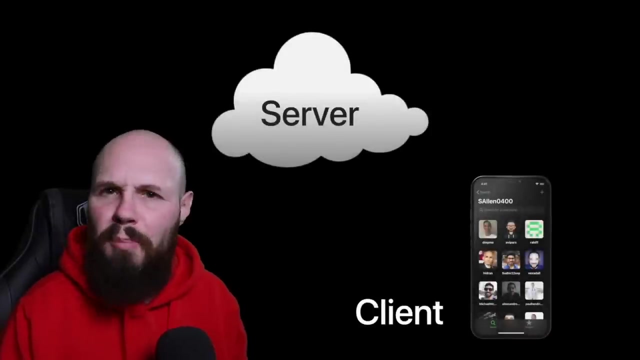 video. now let's talk about what is an api. first of all, it stands for application programming interface, and there's two very common ways that you will use them as an ios developer. the first is for making network calls, as i explained in a previous example, right the twitter and the server going down to the client of the phone. there's an api involved there. 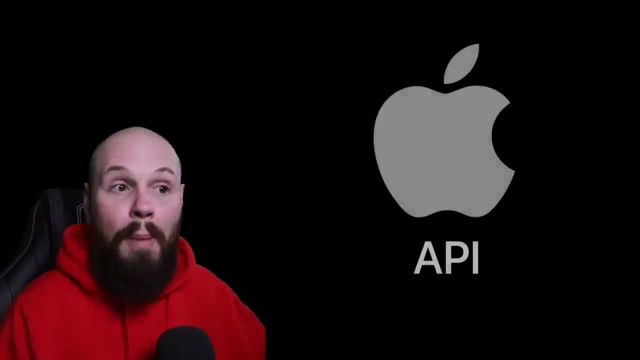 we'll talk about that in a second. and the second way you use them is apple's own apis, right, like we talked about earlier in the course, how you know, apple's laid down this foundation and we're building on top of that foundation. well, how we interact with that foundation is via apis or the. 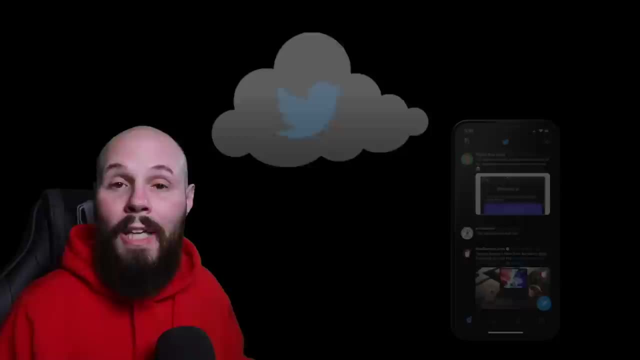 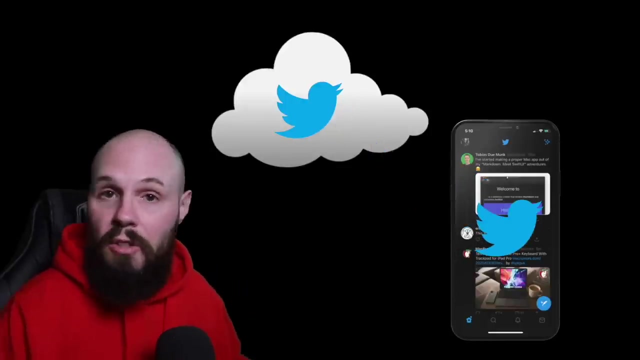 application programming interface. let's dive into those two examples. so back to our twitter example. so let's say that our tweets live on twitter server and our client requests the information to give me the list of tweets to show your twitter feed. well, the client doesn't like reach into the 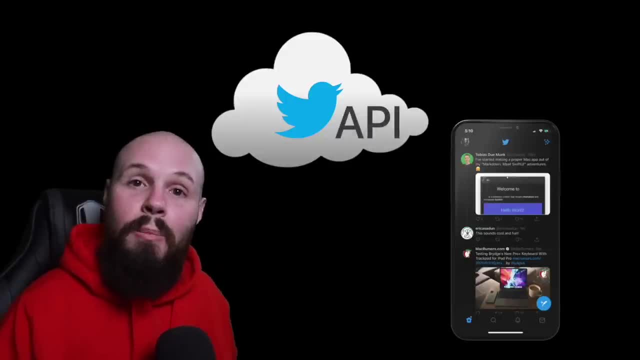 server itself and grab them. the server has an api and the client communicates with the api. it requests information and the api on that server is what handles those requests and also sends the information it needs. so again, our client isn't going directly into the server and grabbing the. 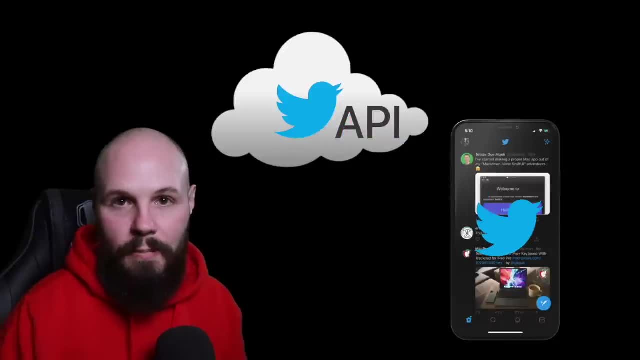 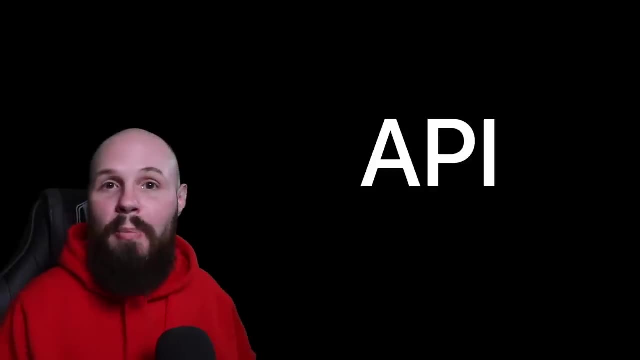 information. the client deals with the api. the api sends back the information to the server and the api is open in the api on the server. they're all over the place. sometimes they're open, like meaning like any developer can access them. sometimes the api is closed, like in. 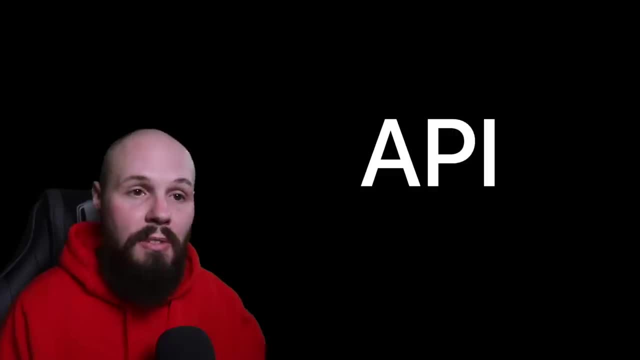 the twitter example. like only twitter developers can access that twitter api for specific stuff. um, sometimes they're free, just open to anybody to use. often those are what's called rate limited, which means you can only send up a certain amount of requests, sometimes it's per second, sometimes it's per hour, sometimes it's per day, depending on the api, but they limit how much you can use it and sometimes apis charge right. they've done a lot of work getting that information and they're gathering this data. they've built their server, they've built their API And if you want to use, 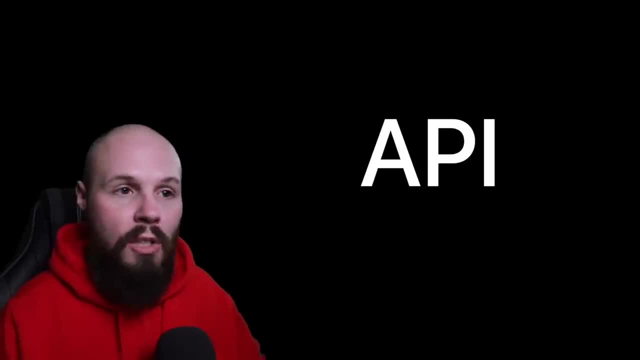 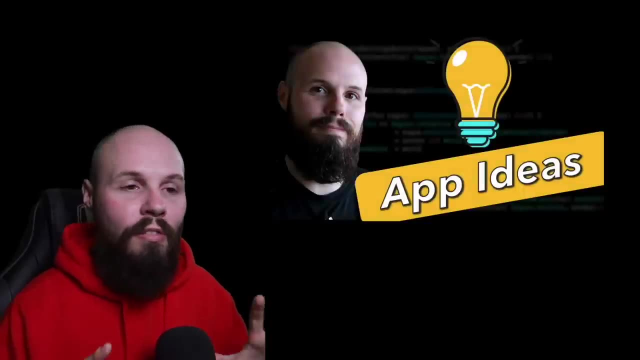 it like you have to pay for it, like per a certain number of requests, typically. So there's a wide variety of APIs you can use. In fact, I'm going to link in the description. there's a resource with a bunch of free APIs. I'm actually going to attach my YouTube video that I did about. 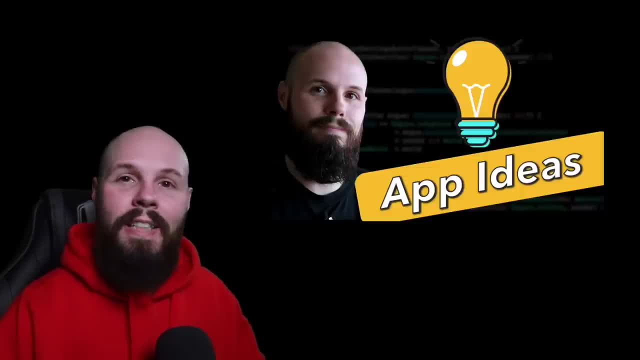 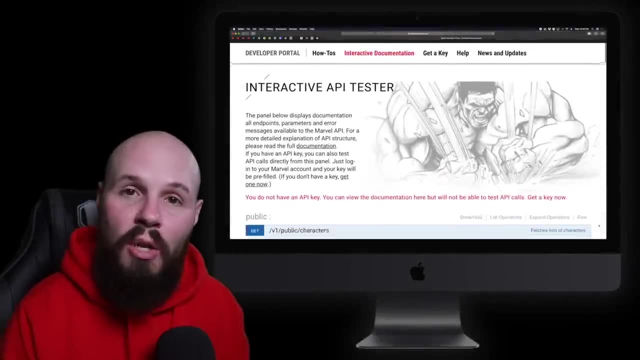 it too on this lesson. So go ahead and watch that video And then check out that link to see a bunch of free APIs. And the cool thing about looking at those APIs is you can get a peek at what the JSON looks like. Remember the JSON was the JavaScript object notation. Well, you can see if you have an. 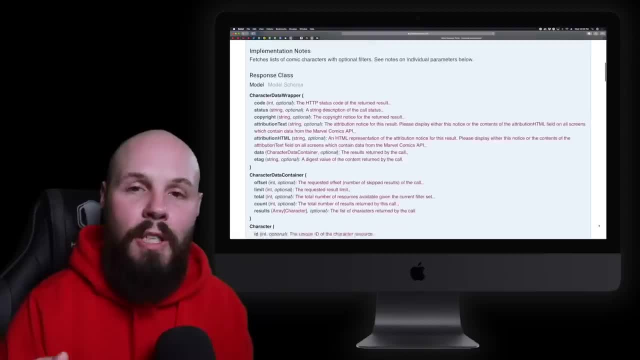 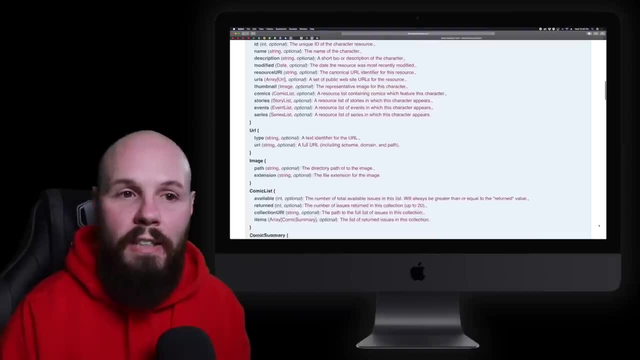 idea for an app. you can kind of see if there's an API out there that will give you the information you need, And then you can even look at the JSON, like, okay, here's what I'm going to get back from this API. Does this have all the information I need? And if the answer is yes, cool, you can use. 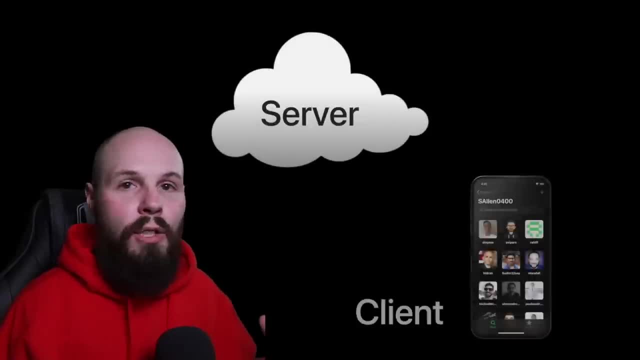 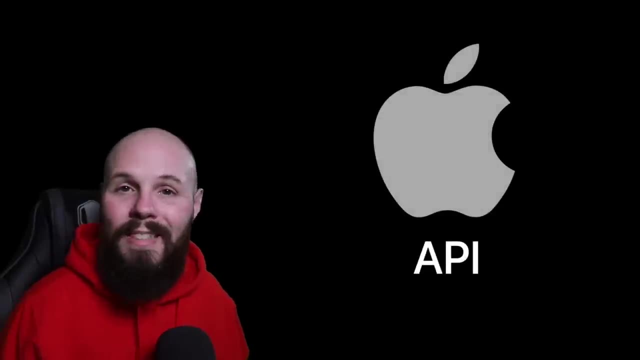 that API and build your app. So that's the example of using the API, you know, as a way to communicate with the server to get information. Now let's talk about the example of using Apple's APIs to build your apps, As I mentioned in the beginning of this video. 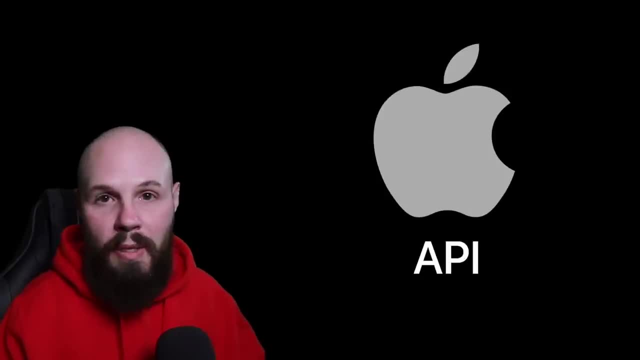 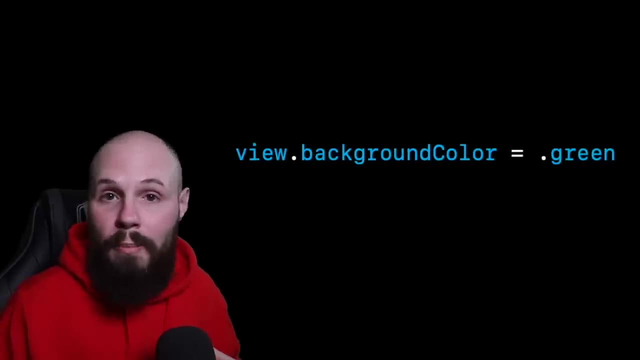 Apple laid the foundation and we interact with that foundation via the API. Like here's an example: right, We can do viewbackgroundcolor equals green. Like that's all we have to do to make a green background. Like we don't have to actually write the code to make the green color. 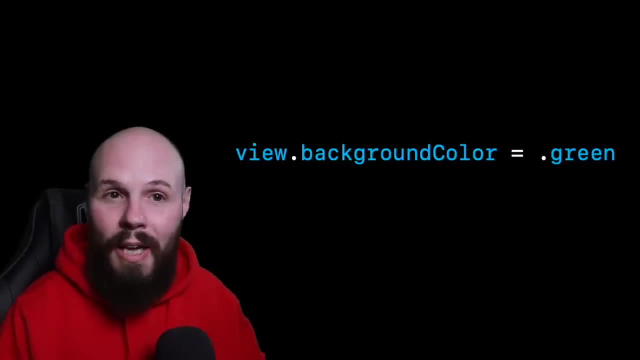 show up on the screen, right. All we have to do is interact with the API saying viewbackgroundcolor equals green, And then all of Apple's code will actually do what it takes to make green show up on the screen, right? We don't actually have to do all that. Another example that we've used: 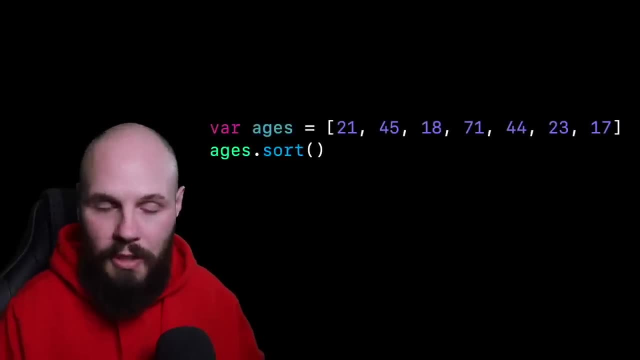 previously in this course is when we sorted our ages array, when we were learning about arrays right. All we had to do was agessort right. That is us interacting with Apple's APIs. We didn't have to write a sorting algorithm to actually sort the array right. That's all Apple's. 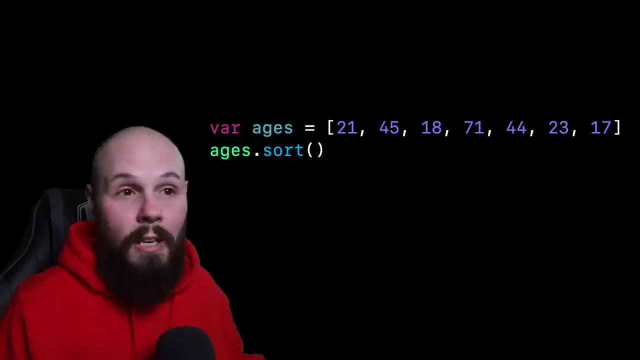 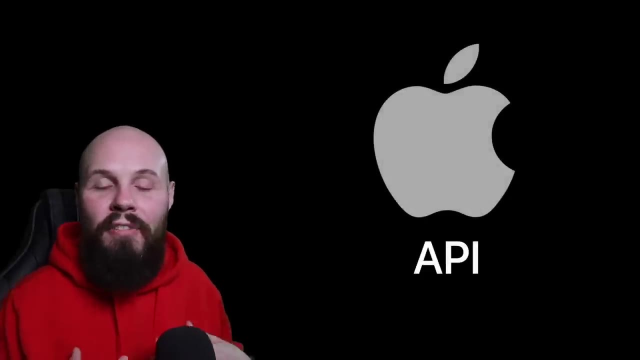 magic code. We're just interacting with their API and just saying, hey, agessort, and we're done. So. those are basic examples of how Apple has done a lot of the heavy lifting to make it very easy for us developers to build our apps. Again, we're interacting with their APIs. 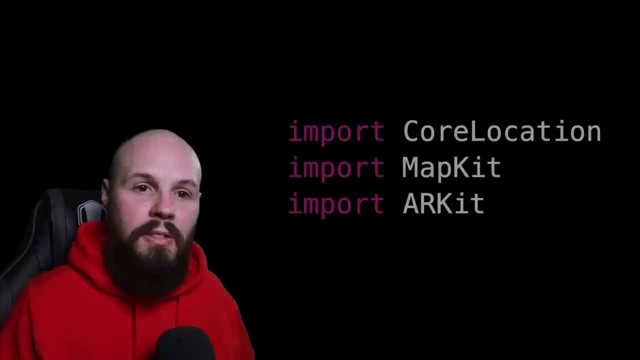 For them to do all the heavy lifting. And all the frameworks have the APIs. right, There's the core location: map kit, AR kit- right, Like these all have APIs that we can interact with. right, When we interact with map kit, we're not building a map. You know what I mean. Like the map's already. 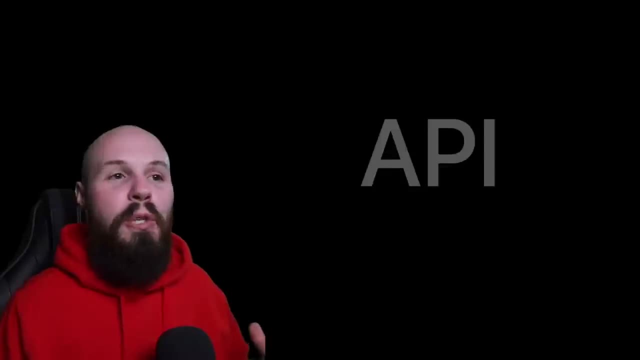 there. We're just interacting with it via the API. So now, hopefully, when you hear a developer say like oh, is there an API for that? Like they're probably meaning the server type API, because they want to know if they can hit that API to get the information they need. Or you may hear an iOS. 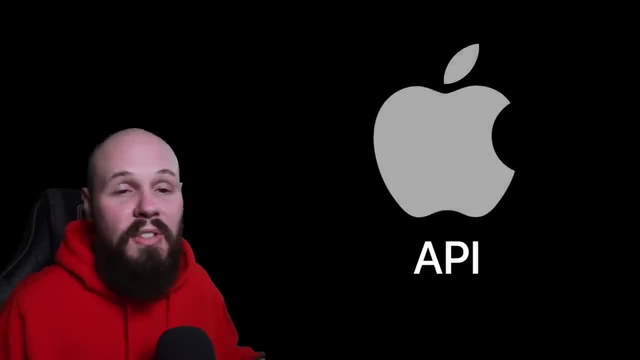 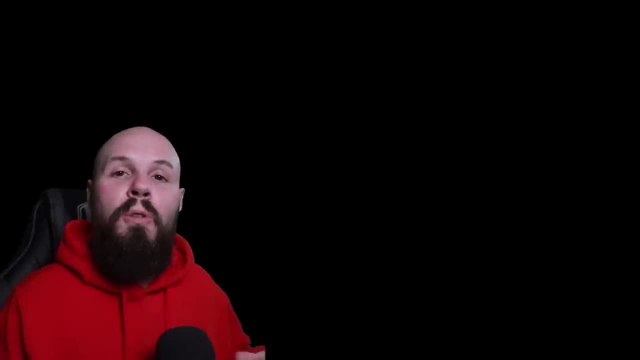 developer say something like: oh, I really love the SpriteKit API, What's that? And they're like what they're saying. is they like the set of tools Apple has given us in order to work with SpriteKit? So, anyway, those are the two most common ways you're going to use an API Again. 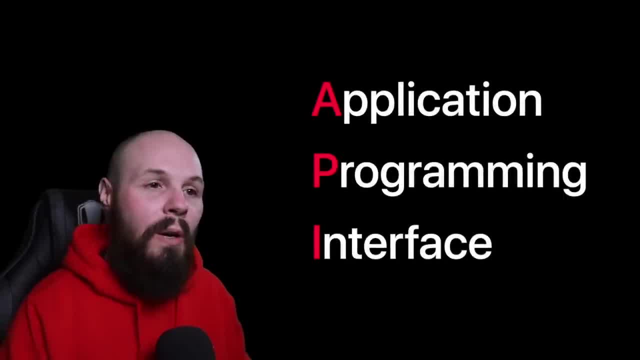 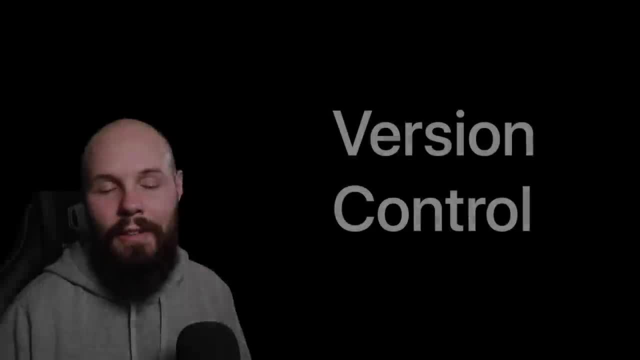 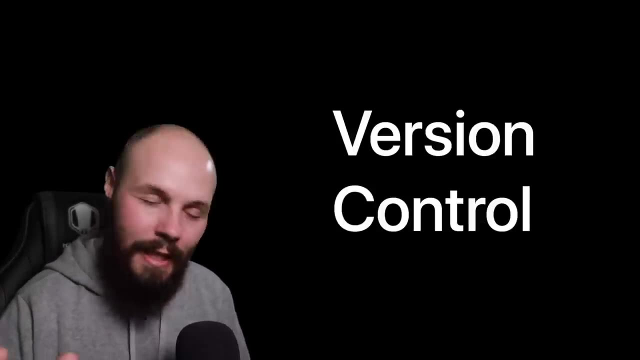 application programming interface- vital fundamental knowledge. Hope you enjoyed On to the next video. All right version control. What is that? Let me preface this by saying this is a big and complex topic But again, as you've heard me say time and time again, we're just. 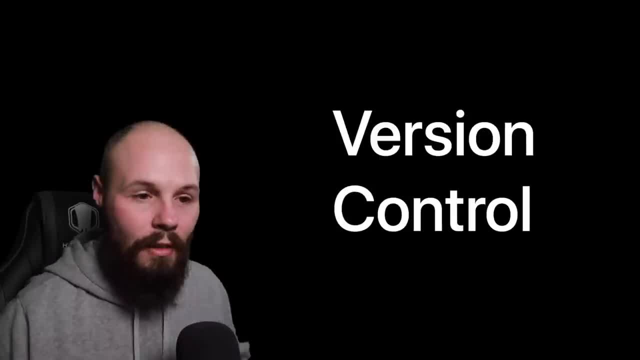 going to scratch the surface, just so you know what it is. So, again, if you feel overwhelmed, don't worry about it. You'll learn much more about this along your journey, But it is a vital skill that you're going to have to know before you get a job and work on a team Because, like I said, 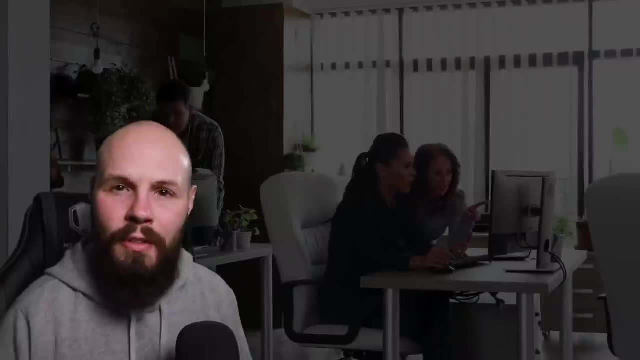 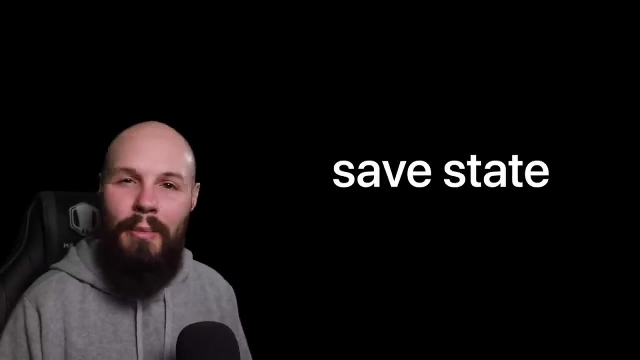 all development teams use this. It's just, it's at the core of development. So what is it? Well, one use is that it's essentially a save state for your code base. Let me use a video game example that I think many can relate with. Do you remember playing a video game and before you got to a big 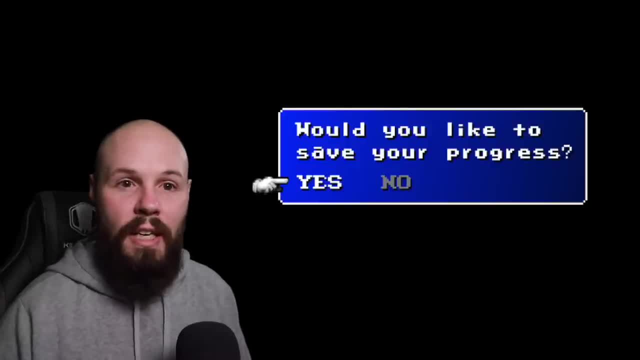 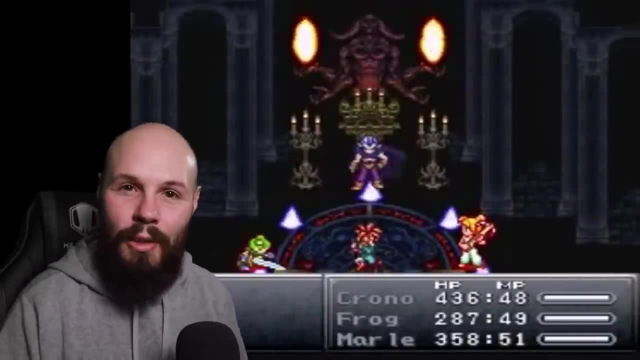 boss or maybe a really hard part in the game- you would save and then that way you could die on the boss, or if you lost one of your key weapons, or if you just really messed up, you could always go back to that save state and try again. That's essentially what version control does with your 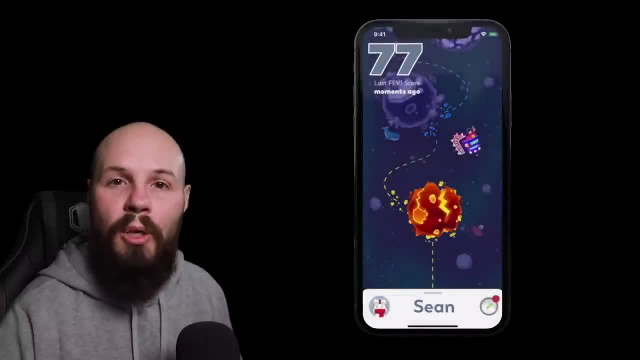 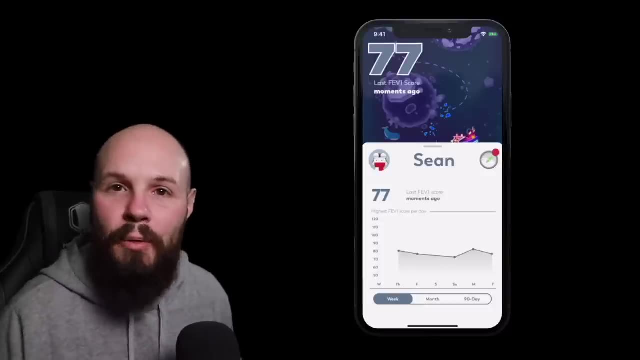 code base. Let's use another example from a Luna like this: this slide up card with a chart like that's a pretty big feature And you can imagine if you're writing code without a save state. like I may not know how to build that feature right away. You know there's probably a lot of. 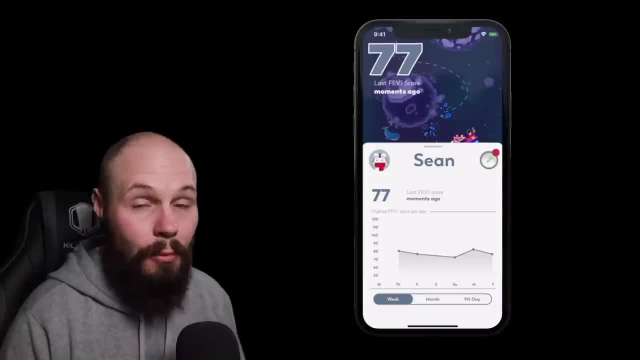 people out there that are working on my code base And I realized halfway through like, Oh man, I really messed this up. Like, how do you unwind that? How do you go back? Well, again, version control can let you like have a save state. So basically, what I would do before building this feature is I: 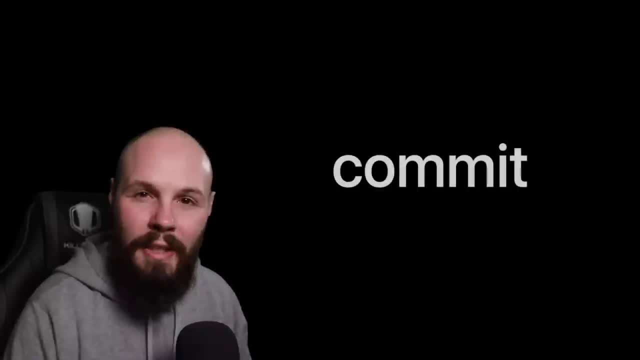 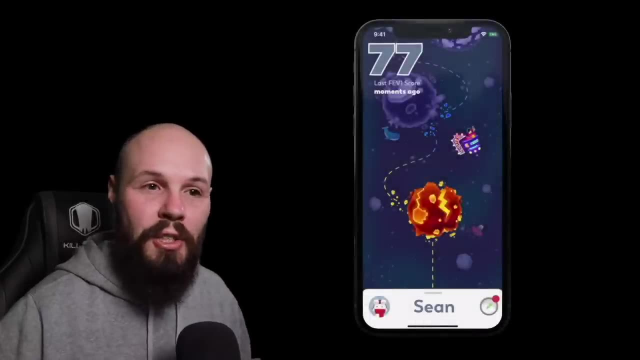 would be like: Alright, let me save my progress right here. There's an actual word for it, called commit. more on that later. But just to keep it in, you know normal people's terms have my save state right before I tackle this big feature. That way, if I just mess up my code base completely, no big deal. 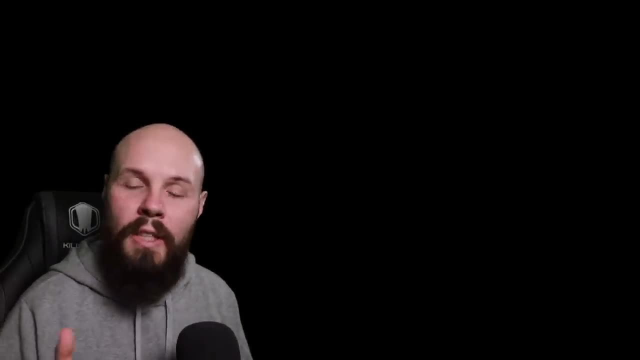 I can go back to that save state right before I started that. So back to that word commit. So that's the, that's the lingo, right? We don't call it a save state. you say, Alright, I'm going to. 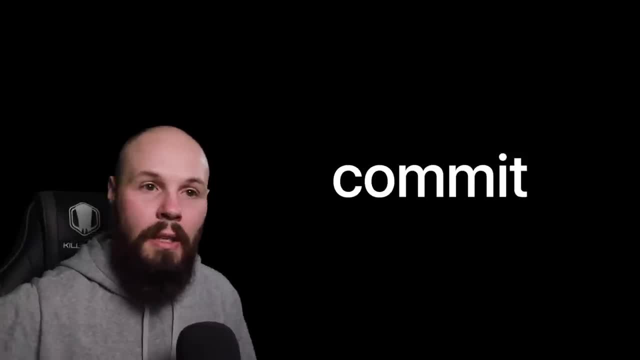 commit my code And then now that's the save state And now I can. I can mess up my code base entirely And I can always go back to that commit. The cool thing is is you're making a ton of commits all. 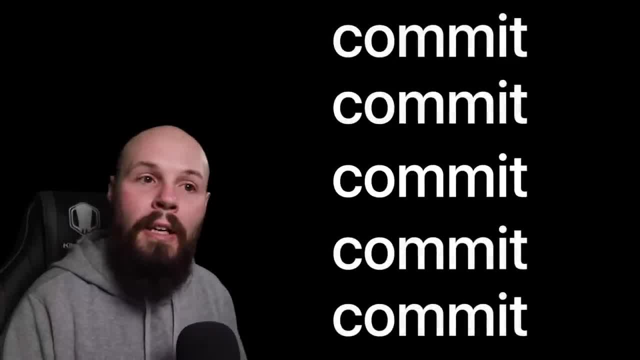 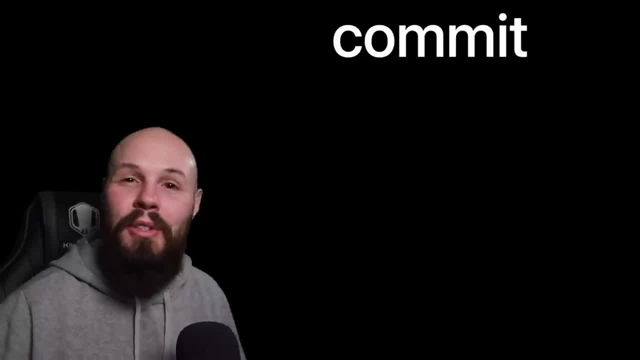 throughout your code base as you're building your product And you can go back to any commit, right, so you can unwind it back to six commits before like again, let's say you know you've written this huge feature and you've been committing along the way. 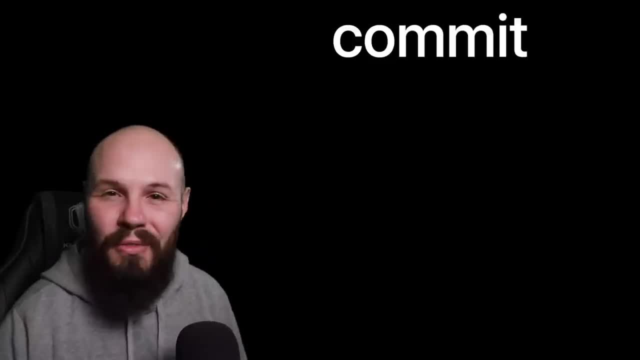 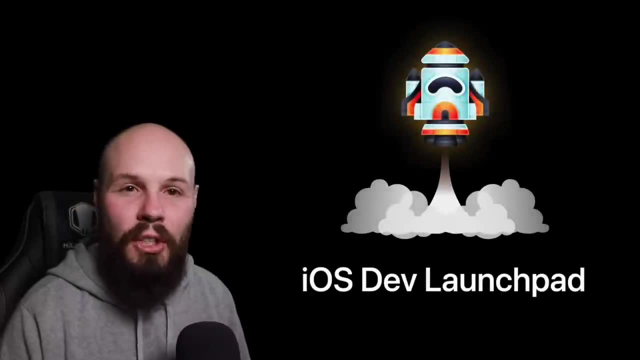 and then you realize, oh crap, I messed up or maybe we don't really want this feature Again. you can go back any number of commits to specific save states And that's a nice insurance feature, because I know when I first started coding I was so worried that I was going to 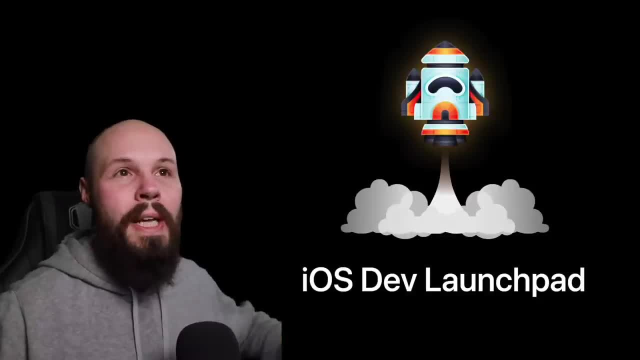 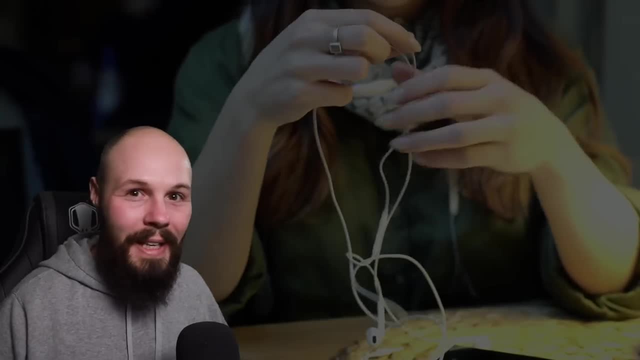 mess up the code base, like I was going to break it. Well, the beauty of version control is, for the most part, like you can't break your code base because, again, you can always unwind it. Don't get me wrong: sometimes unwinding it and doing all that stuff is a giant headache. 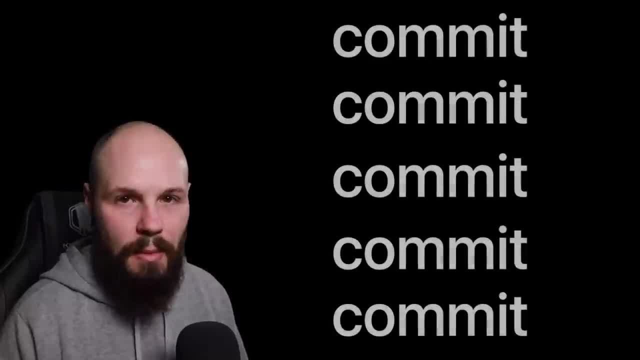 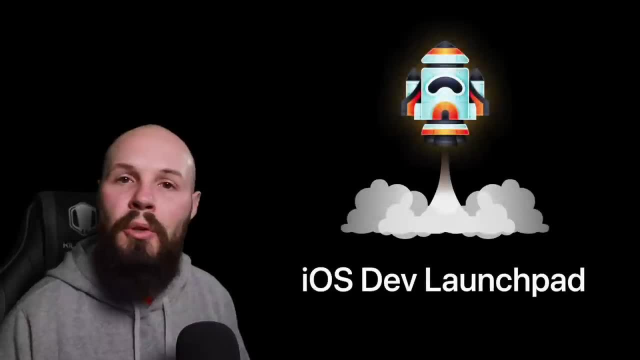 But for the most part it's always possible. So that was a very simplified example of you know, keeping safe states of your code base along the way. Now let's talk about how development teams use this to build their products. right, You ever? 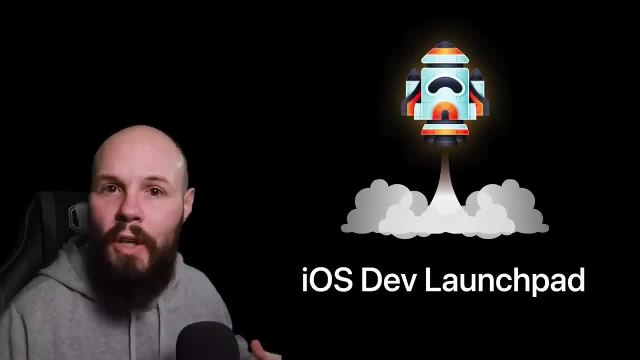 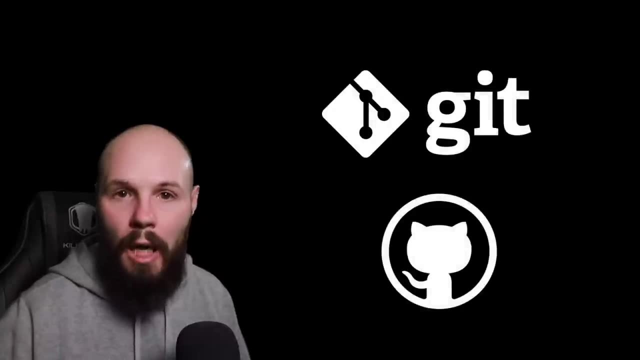 wondered how big companies have development teams of 10 to 20 developers all working on the same code base and how all that works. Well, let's talk about that. Let's talk about Git and GitHub. Maybe you've heard of these things First thing, and I didn't know this for a while, but, like 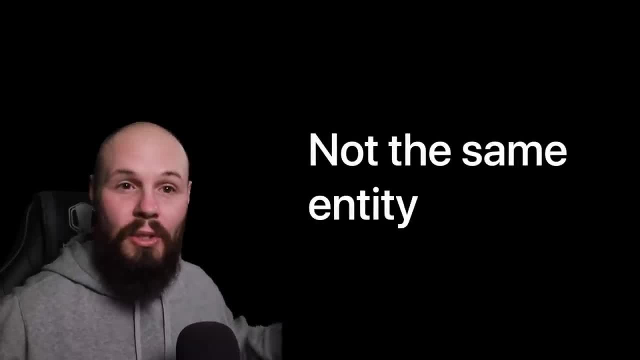 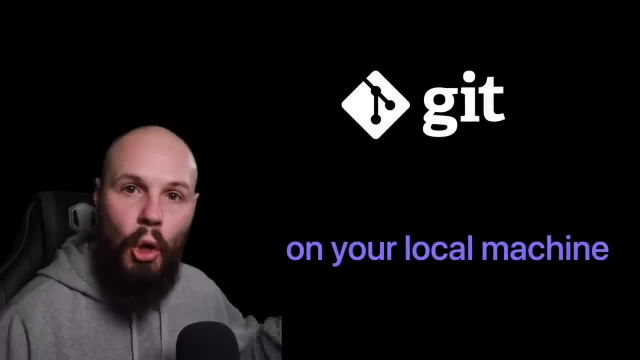 Git and GitHub are not the same thing, So let's talk about what they are. Git is version control on your local machine. Let's define some terms real quick too: Local and remote. Local means it's on your computer, right, Anything you have locally. let's say you threw your. 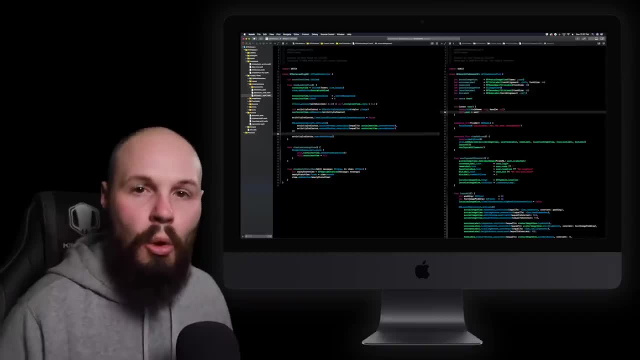 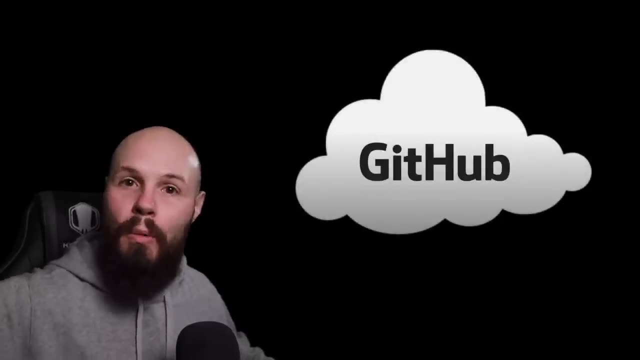 computer into a lake. Well, you're going to lose all that data because it was locally on your machine, Whereas remote lives on a server somewhere. So you could throw your computer in a machine but you got your code base remotely up on a server. so just buy a new. 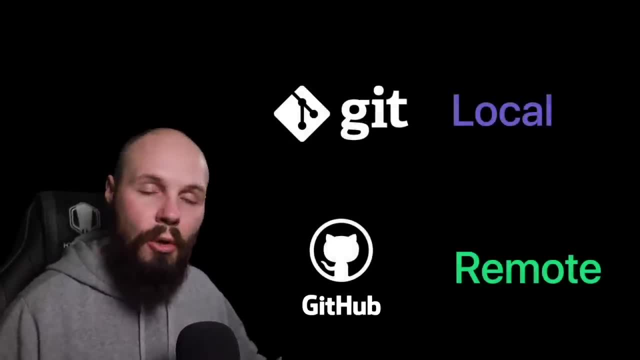 computer and download that code base and you're good to go. Okay, so that's local and remote. And again, Git is the version control on your local machine is an online server to put your git repositories up on the server and real quick. there are other. 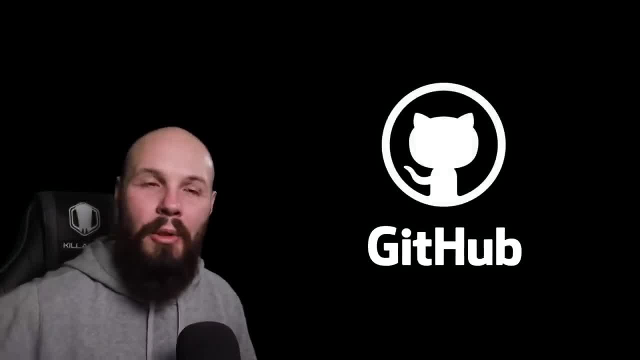 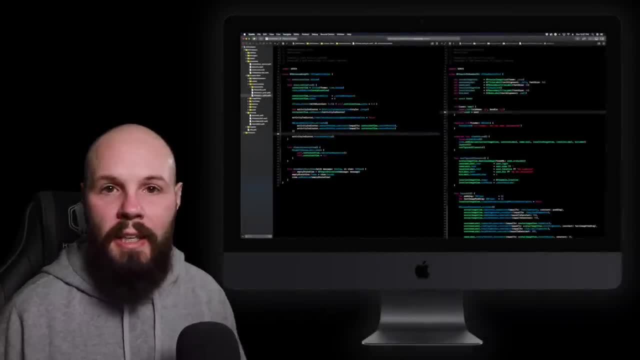 services like bitbucket that kind of do the same thing as github. those are kind of niche. github is the dominant player in the space. so a simplified example of how development works with git and github: i'm writing my code base on my local machine. i build my feature or my save state, my 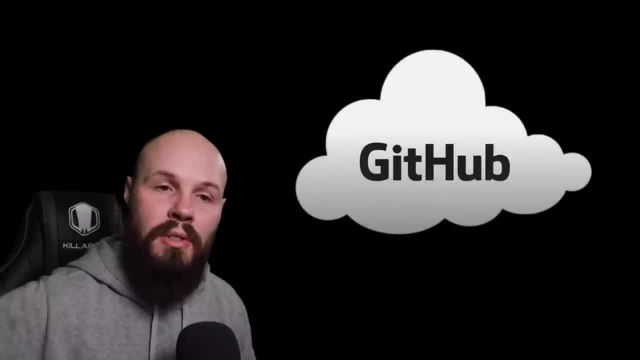 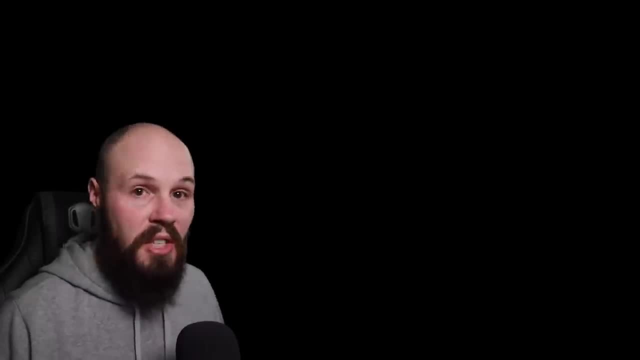 commit. i want to send that commit up to github so it lives on on the remote repository. and again you want it on that remote depository. that way you can pull down that code base on any machine, right, say, you have a work laptop or a personal laptop or you're working between a laptop and a. 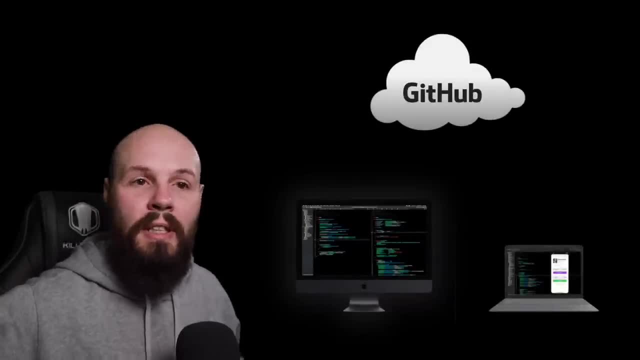 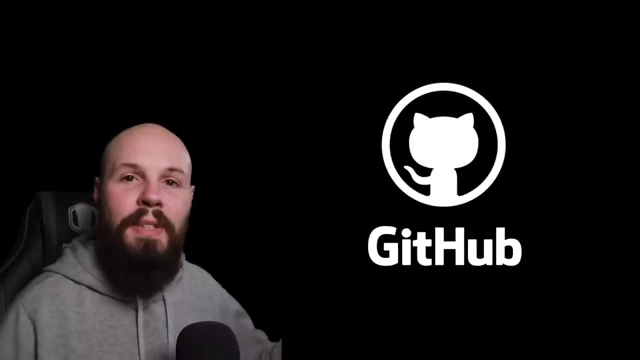 desktop computer. it's all the same, right, because the code base lives remotely in the cloud and you can pull that down to any machine, right? and that's what github does. github stores those repositories. now let's talk about how development teams use this to collaborate on one project. now again, i'm 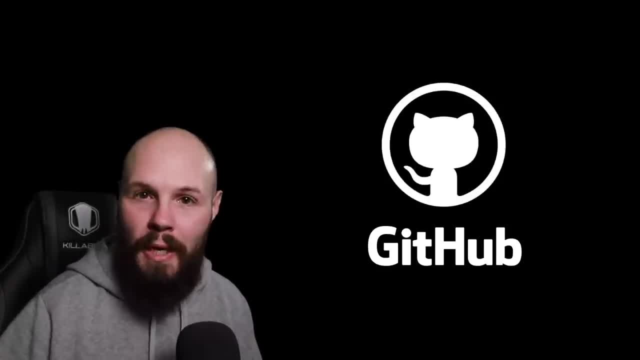 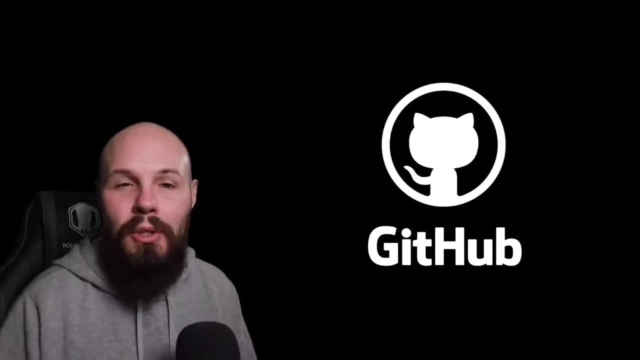 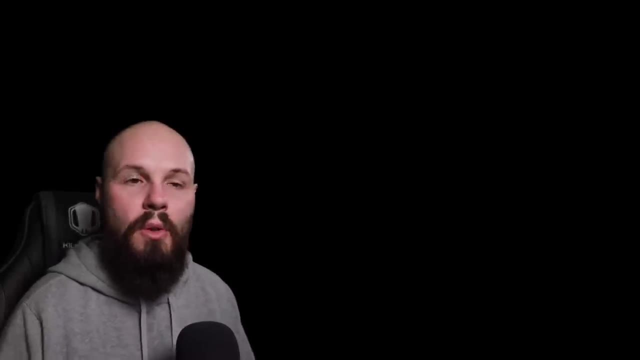 going to give a very simplified example, because this can get very complex. like i said, you have development teams of 20 to 50 to even 100 people working on one code base, so you can understand that that can get very, very complex. but again, just the simplified version, just so you have an idea of how it works. here we go, so. 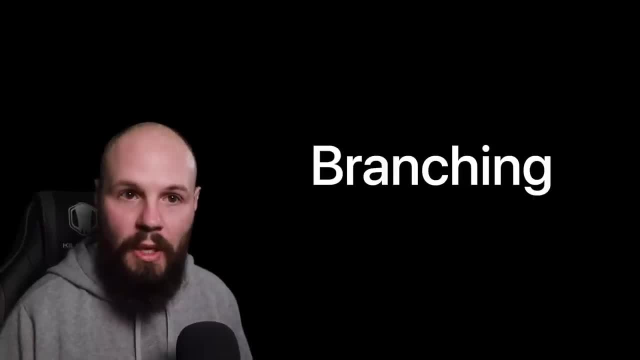 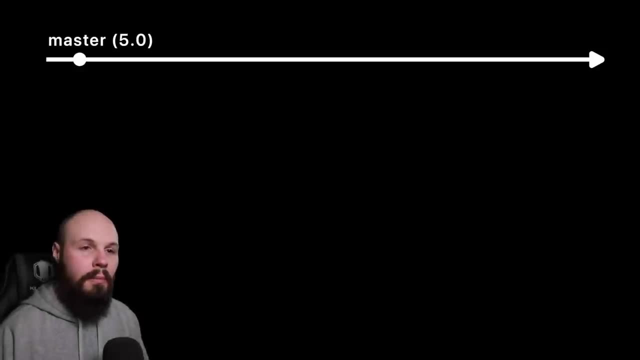 the power of git is a concept called branching. so let's walk through a visual example so you'll understand this. so typically, you have a master branch and let's say we're working on the version 5 of twitter. so on, this master branch is always the version that's on the app store, and the reason 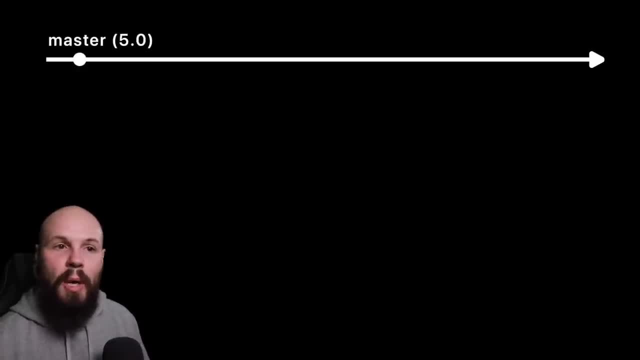 you want that is because, if a master branch is always the version that's on the app store, and the reason you want that is because if a user has a bug, or bugs pop up, you want to be able to go to the version of the code base that the 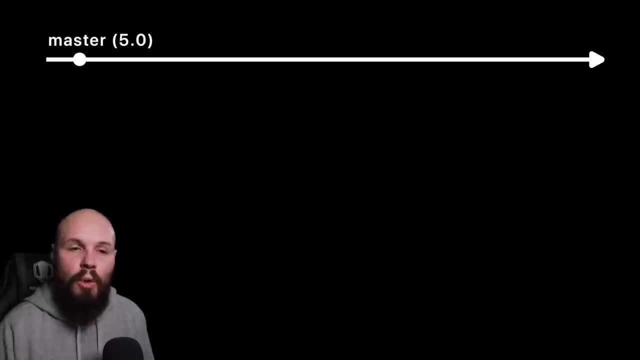 user are actually using, so that's typically master. now, of course, we're on version 5. we want to eventually get to version 5.1 or 5.2, so we need to be able to work on the code base but not affect the master branch that the users are actually using. so this is again where you branch off of. 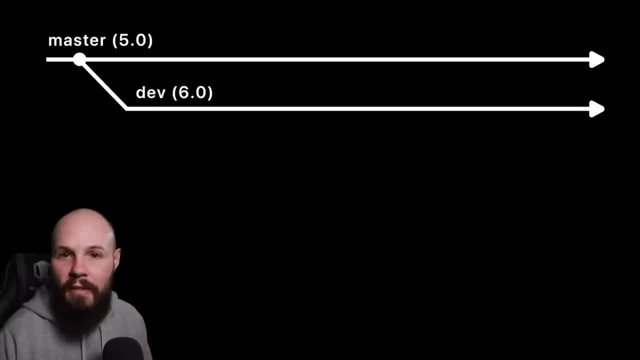 master. and again, typically the first branch off is called something like dev or development. so again the very simplified example: we branch off development, we do all of our work on development that is going to go into version 6 and then, when version 6 is ready, we 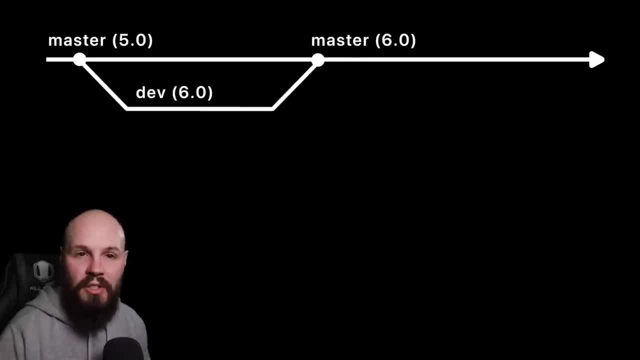 merge development into master. now master is on version 6 and that's when we push that version to the app store. and now the version 6 is on the app store. that's what the master branch is, and then we continue that cycle all over again. for version 7. we got to branch off onto dev, do all. 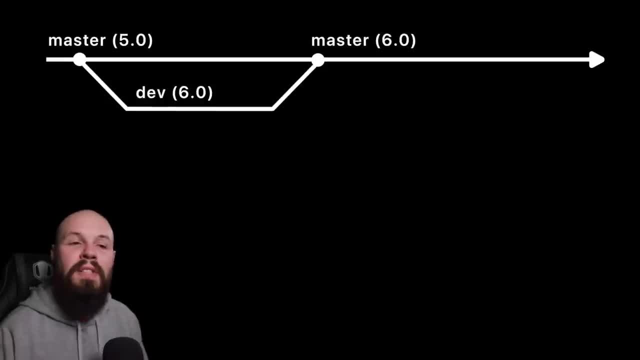 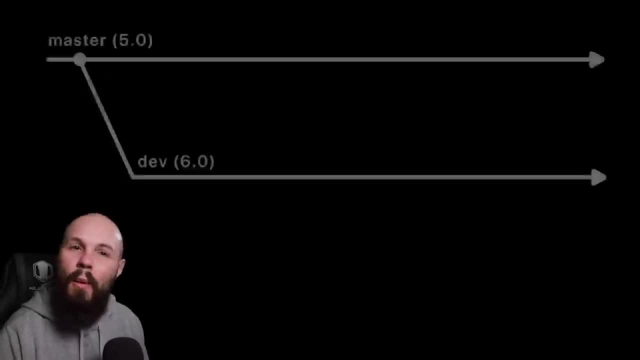 of our work, merge it back in for version 7. now let's expand on this example a little bit, because i just kind of, you know, wave my hand over what was going on on the dev branch. let's actually zoom into the dev branch and talk about what happens between version 5 and 6. right, because remember. 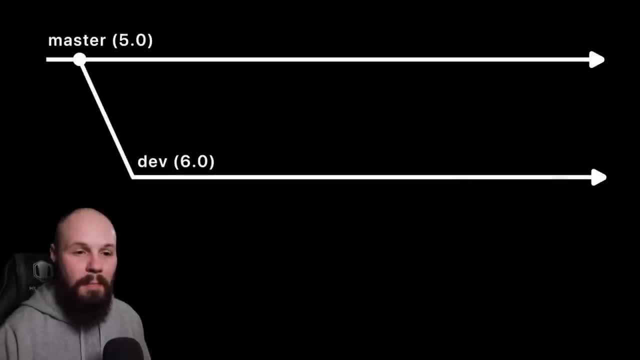 i just said we do all of our version 6 work and then we merge it back in. well, let's zoom in on that now. remember we talked about working on a team, so different developers can branch off of this dev branch. so let's say i want to build a feature where i'm building the chart and another. 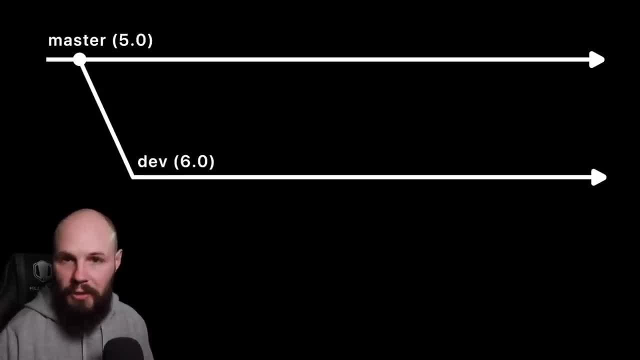 developer wants to build a feature where they're implementing new changes to the profile screen. so once we have the dev branch, i will branch off of dev to build all the chart stuff and my teammate, the other developer, will also branch off of dev to do the profile stuff. now, maybe their change was a lot more fast than mine. 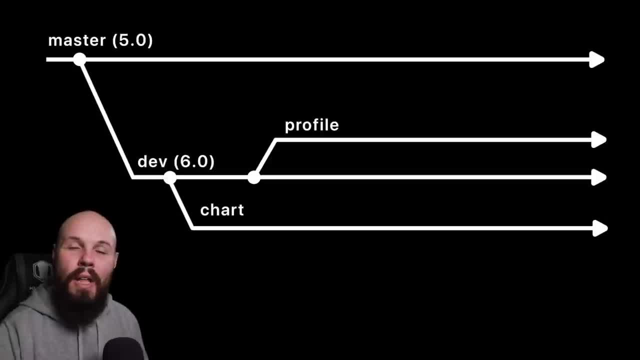 right, i'm building a whole chart. they're just updating the profile screen, so they would have their fixes and they would merge back into dev, like you see here, and i'm still working on mine, but, as you can see, dev has changed since i branched off of that. so what i can do is you know. 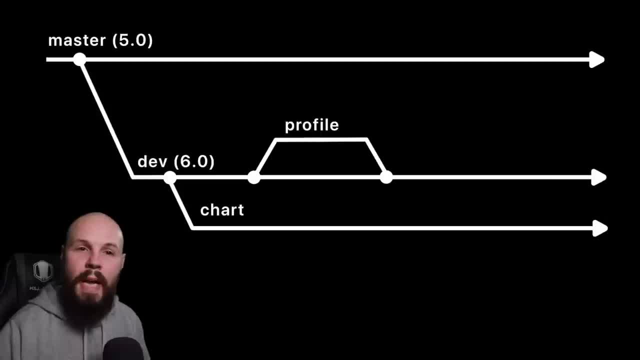 my teammate will be like: hey, sean, i finished my profile work. i merged it back into dev. if you want to pull down the latest dev into your branch, that way you can have all the changes. so what i can do is i can pull in the latest version of dev into my branch and keep working on my own branch, but that 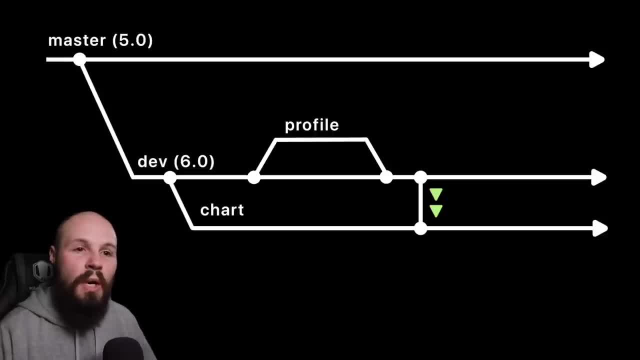 ensures that i have the latest version of dev now. the reason you want to do that is, as you can imagine, like: let's pretend you know my feature is huge. it's going to take me two months to build so i'm on my own- my own branch. well, dev is constantly being worked on, so dev is going to change a lot. 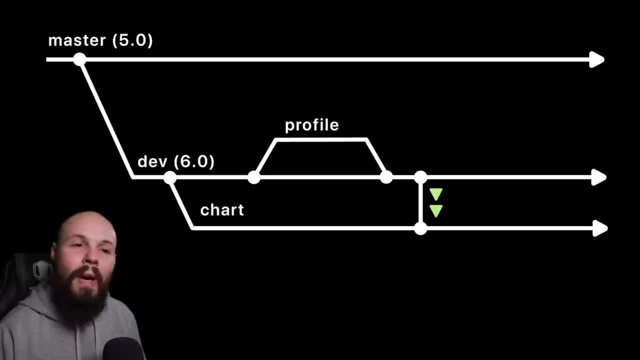 before i'm ready to merge my changes back into dev. so that is why i want to constantly be pulling in the new dev into my branch to make sure i'm up to date and i'm not like breaking anything. also, what there is something called merge conflicts- you may be thinking this already if you have multiple. 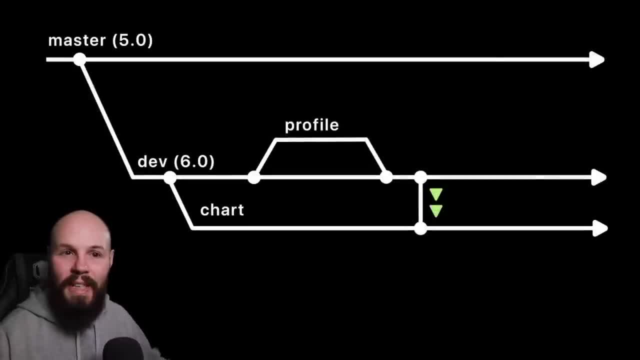 developers working on the same code base and then you try and merge it all together. like what if you were working on the same you know screen in the same line of code, like whose, whose changes you know get merged. well, merge conflicts can be a headache, and they do happen with teams. good. 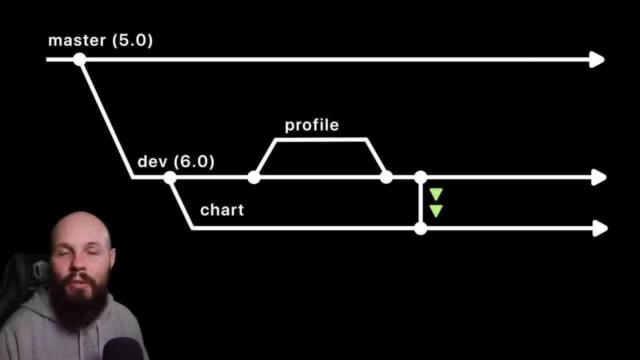 communication on, like, what section of the app you're working on is a good way to avoid it, but that can happen. so, again, that's another benefit of consistently bringing in the dev branch into my branch. so if there are merge conflicts, they're likely to be small and easily fixable, whereas if 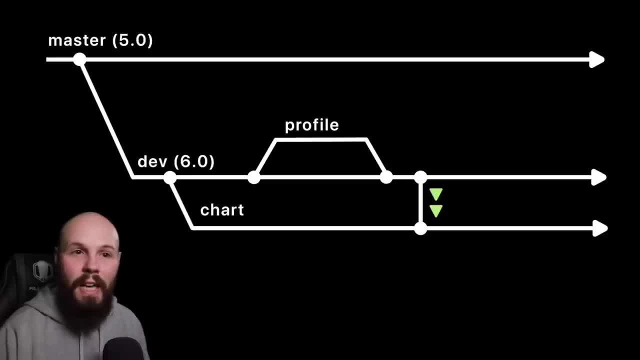 i just worked by myself for this long time on the dev branch and then two months later tried to merge my branch back into dev. dev is going to have changed so much. very likely there's going to be a lot of merge conflicts and it's going to be a headache to untangle. all right, i worry going on. 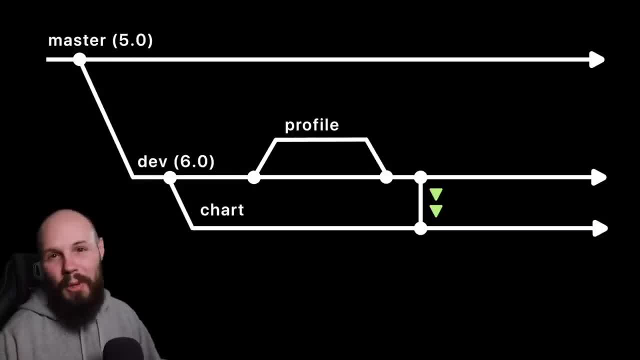 that merge conflict tangent might have been overwhelming. don't worry about merge conflicts right now as a beginner. you're going to deal with that way later in your journey. but again, just know that they exist. and back to how these branches work. eventually i'll merge my changes into dev. the other developers. 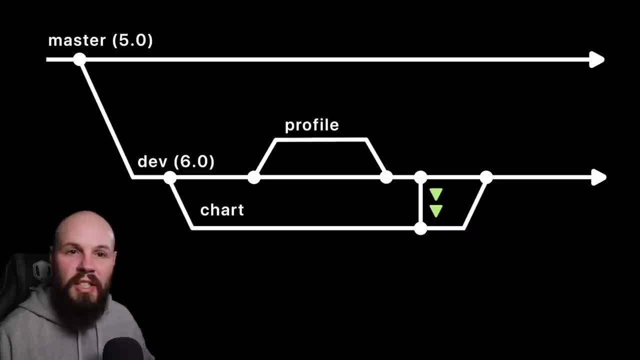 will merge their changes into dev. the team will say, okay, great, version six is ready. and then we merge dev as a whole back into master for version six to push to the app store. so that's how a team of developers from all around the world can work on the same code base. right, because the code base 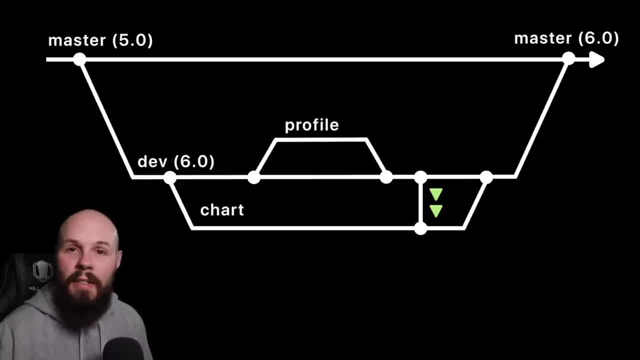 lives on github, on the remote server. so, like i said, my teammate could be like: hey, sean, i push my code base on github and i'm going to merge my changes into dev. so that's how a team of developers changes up to the dev branch, he pushes them up to remote and i can be living across the world. 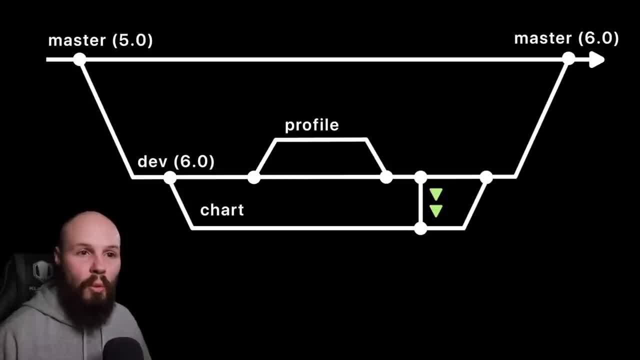 and i can pull it down- his changes into my computer to work on the latest version of the app. now again, these were all pretty simplified examples. like i said, a team of 20 to 50. you can imagine how this can get pretty complex. but again, at least you know this exists now, if you are. 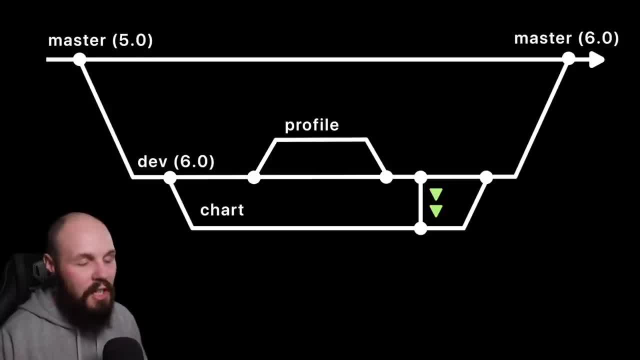 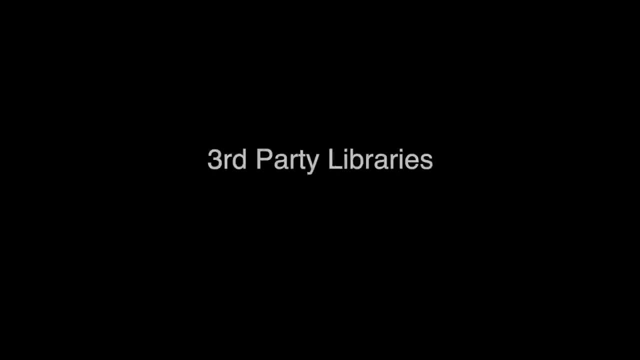 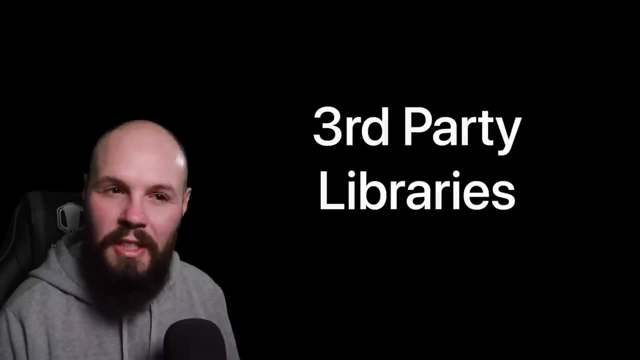 confused. that's perfectly fine. this is a confusing topic comment section, as always- and then feel free to hit up the slack channel to ask questions about it. everybody in there is more than helpful. see in the next video let's talk about third-party libraries, or you may hear them called dependencies. 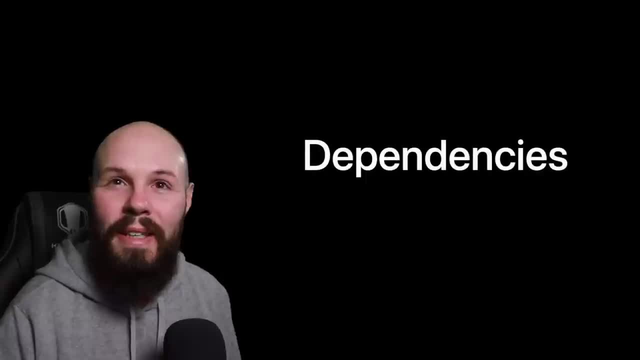 or just libraries, it's all the same thing. what these are is basically a module of code that other developers have written that you can bring in and use into your code base. let me give you an example here. in the aluna app, we track the user's measurements via a chart that you can see here. 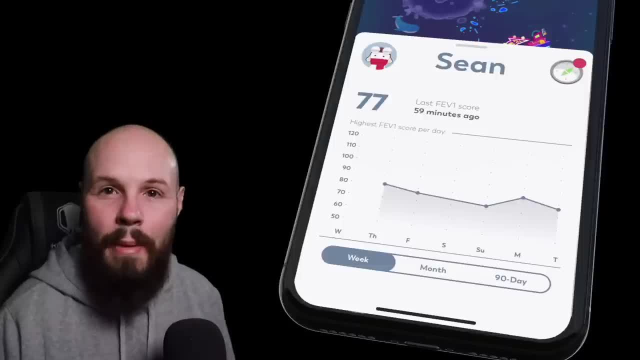 now creating a whole line chart that can be flexible and dynamic and take in different date rates and different time periods can be used to measure the user's measurements, and then we can create a chart that can be used to measure the user's measurements, and then we can create a chart. 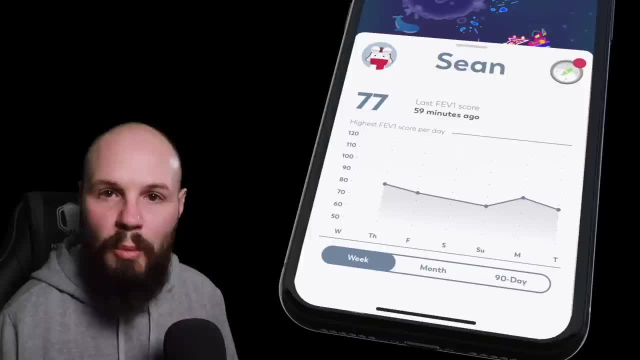 ranges. that's a lot of work. so in this case, we brought in the third-party library called charts to help us make this chart. now, of course, you can customize it as you can see. the colors match the app, but the core foundation of building the chart was completed by the library. these libraries are: 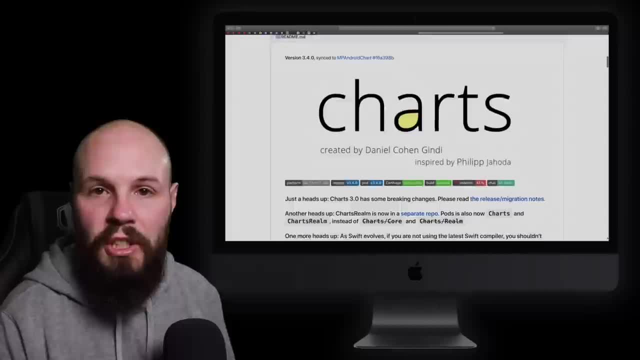 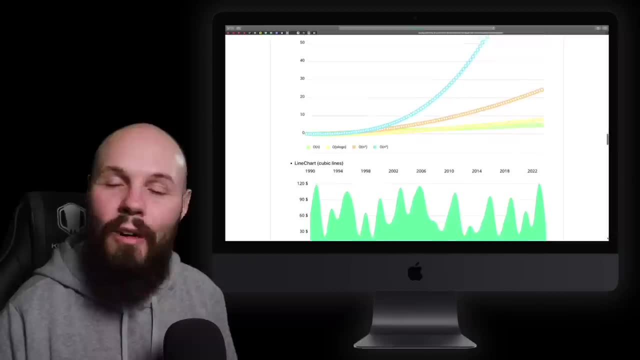 often hosted on github so you can go check them out. so, for example, here is the charts library. it'll show you how to use it, it'll have the documentation and even some pictures- hopefully, if it's a good one- of what it does. so, as you can see, there's various different types of charts in this. 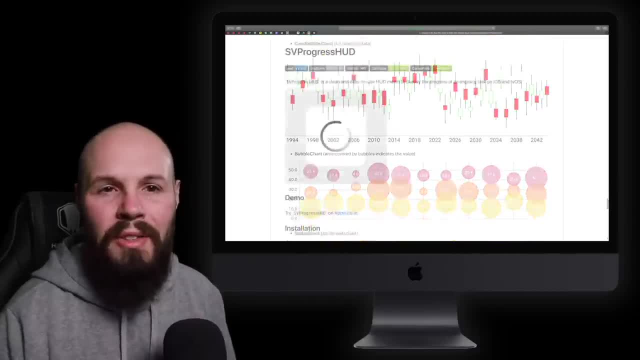 library and just to give you a little bit of an idea of what it's all about, let's go ahead and just give you a couple more examples of what you can do with libraries. you know, here's a progress hud. here we have some different transitions you can do via view controllers, and then there's other. 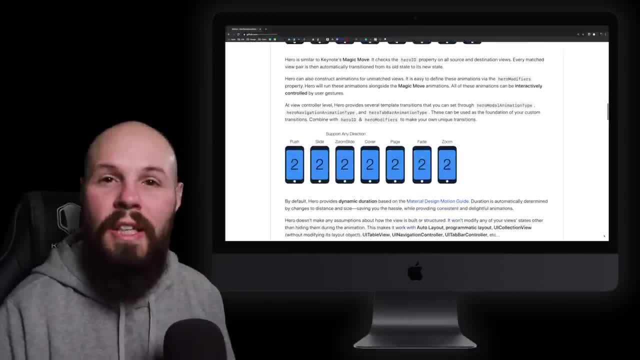 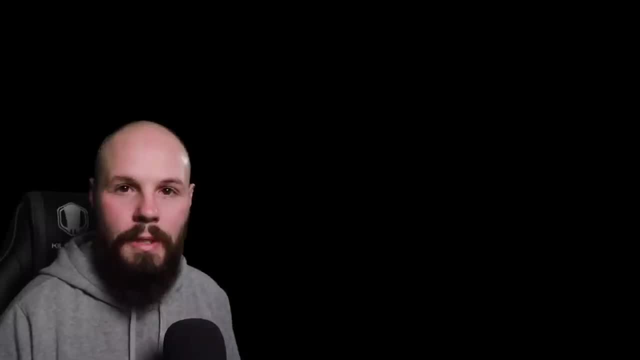 libraries that can help you out with, like your networking code, you know, to talk to the server and the client, and there are a ton of libraries out there that you can use. but that's where you got to be careful. but we'll get back to that later in the video. let's talk about how you go about. 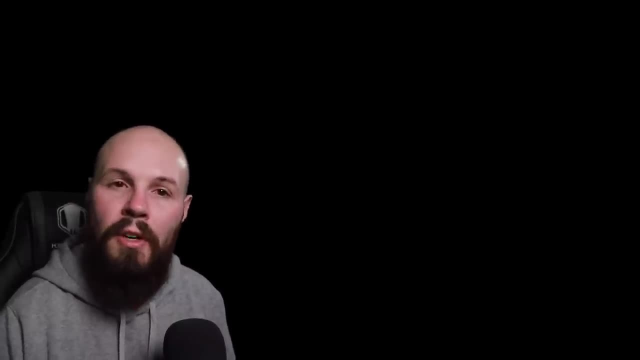 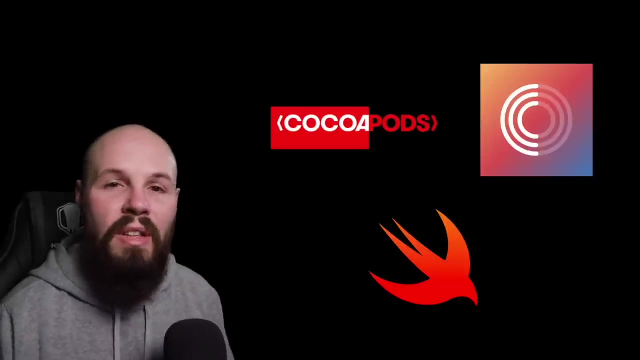 using these libraries, because you may have heard these words before. right, you may have heard: coco, pods, carthage, swift, package manager. those are what you would use to install these libraries. now let me give you the lay of the land real quick, because this area is changing. 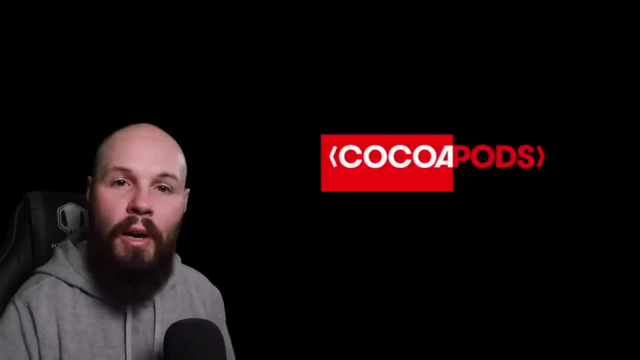 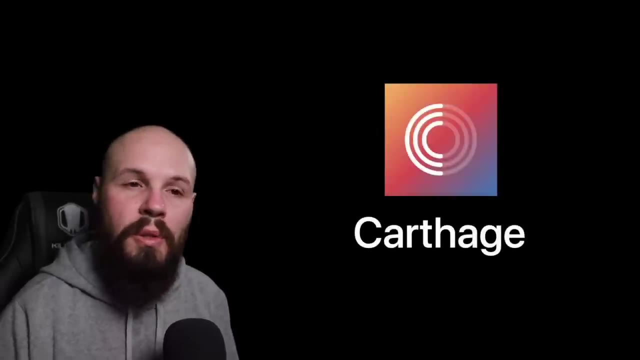 as we speak. right, coco pods is the incumbent. they've been around for for years. this is the. this is the main way people install their libraries in ios development. and then carthage came along a few years ago and was kind of a competitor to coco pods. however, swift package. 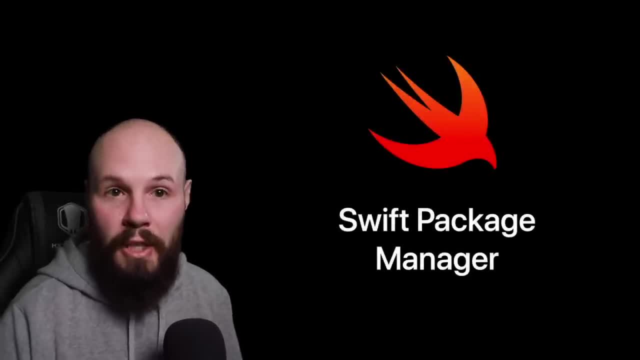 manager. that is apple's first party dependency manager and that just came out, i believe a year or two ago, so that is still pretty new. but even though it's new, it's rapidly gaining popularity amongst developers and, in my opinion, in another year or two, swift package manager is going to be. 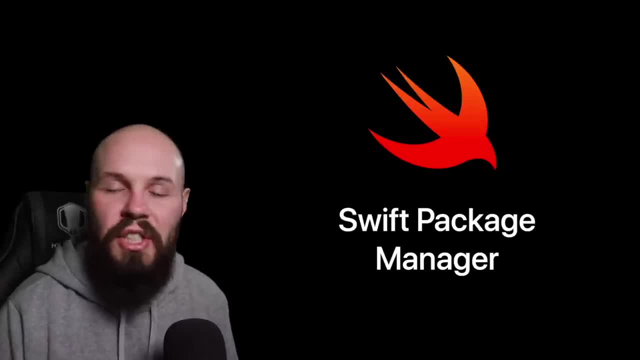 like the default way all developers do it. we're kind of in a transitionary period, so the advice to you, just learning, is when you do decide to tackle these third-party libraries again. i don't recommend it for beginners. don't worry if you don't fully understand all this now. this is more. 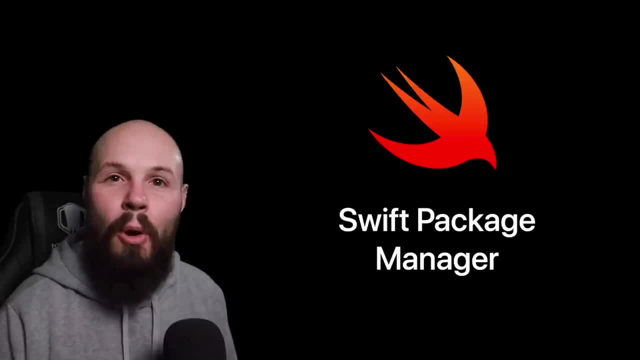 for later in your journey. but just remember when it comes time to third-party libraries. you're going to see a lot of information about coco pods out there because, again, they were the incumbent for so long. but swift package manager is what i've been using for a long time and i've been 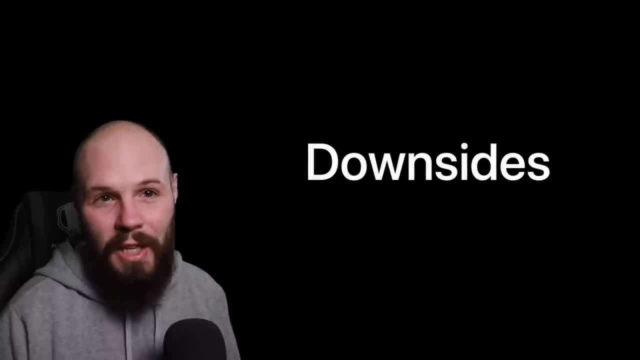 using it for a long time and i've been using it for a long time and it's been a lot of fun to work with and i've been using it for a long time and i've been using it for a long time. so let's talk about those downsides, because i know you may be thinking, wow, if there's a library. 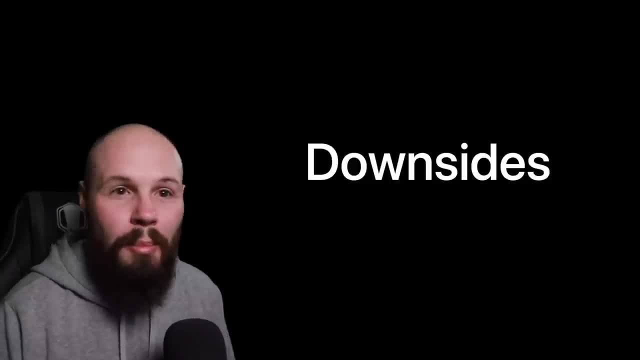 for just about everything, man, i can just find a library, put it together like a puzzle and there's my app and i get your logic. i understand that and that's how a lot of web development is, but uh, i wouldn't do that in ios development. the general rule of thumb is that using libraries is 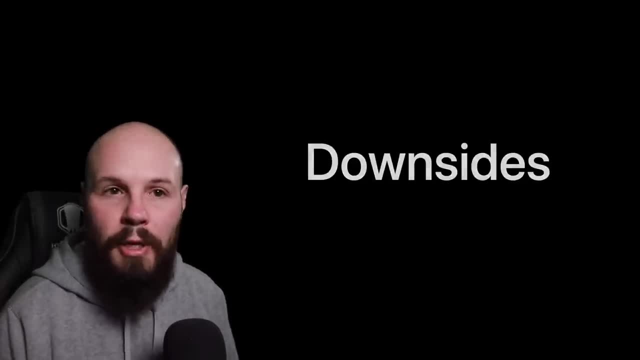 okay, but use them sparingly, and here's why, right, they're called dependencies for a reason. you're depending on other people's code and, as you may have noticed, in the past year i've been using the word dependencies for a reason. i've been using them for a long time and i've been using them for. 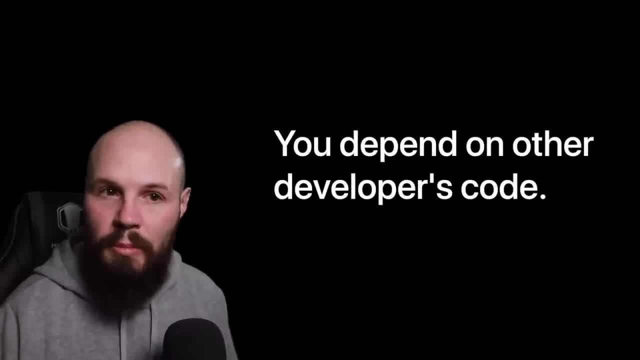 may know, may or may not know. Swift is a rapidly evolving language because it's only five years old, it's still kind of growing. and also the iOS platform- uh, constantly changes, right, iOS 13, iOS 14, the, the new phones with the notch. so the platform and the language are constantly evolving, which is 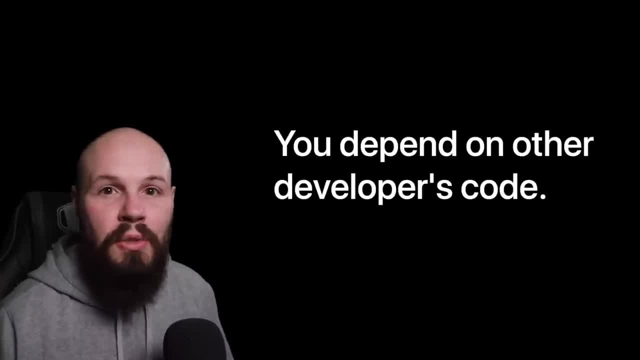 fine. that's actually what I like about it. but if you find yourself using 20 libraries now, you're counting on those 20 developers to keep their library up to date and, trust me, it is very, very common for libraries to get abandoned and no longer maintained. like you'll go to it and it'll. 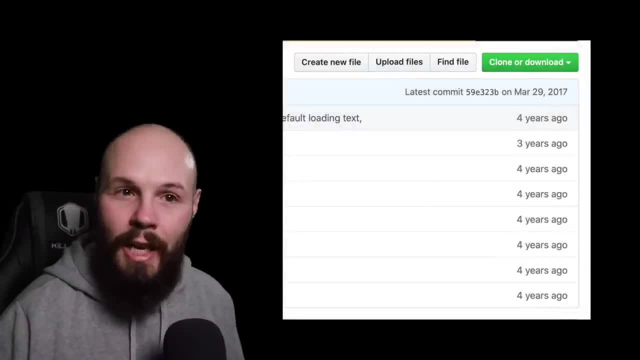 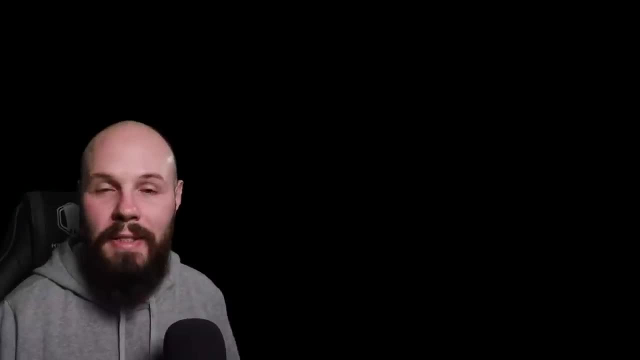 say, the last update was two years ago. well, you know that's pretty much a dead library. so not only do you have to use them sparingly, you got to be careful in which ones you used to make sure that they're actively maintained. now the good news is the most popular ones like this, chart ones as 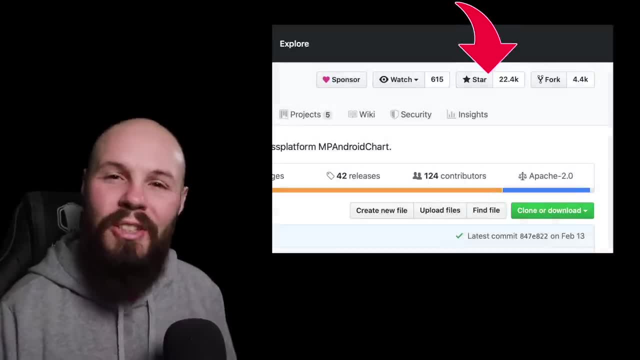 you can see here, you always want to look for the stars on the github repo. that's a good indication of how popular it is, which is a direct proxy to how much it's used. so the more it's used, the more it's apt to be, you know, actively maintained. 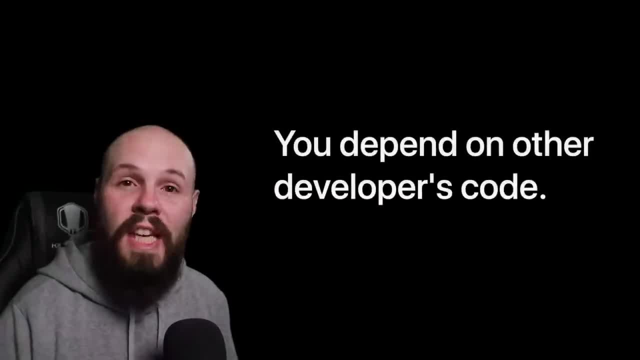 because, again, if you're relying on a library for a key piece of functionality in your app and then all of a sudden that library stops being maintained, now you're stuck with this old code and as Swift updates, as iOS updates, now you have to maintain it yourself or find a different one, and again. 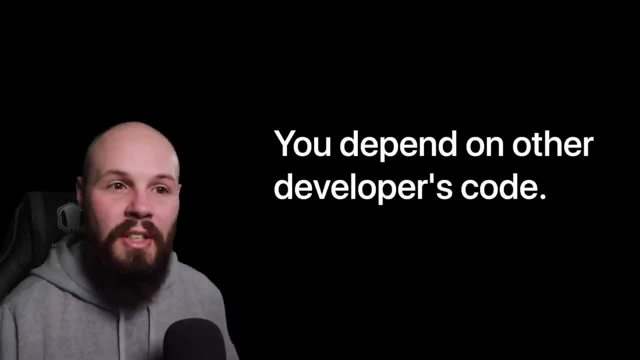 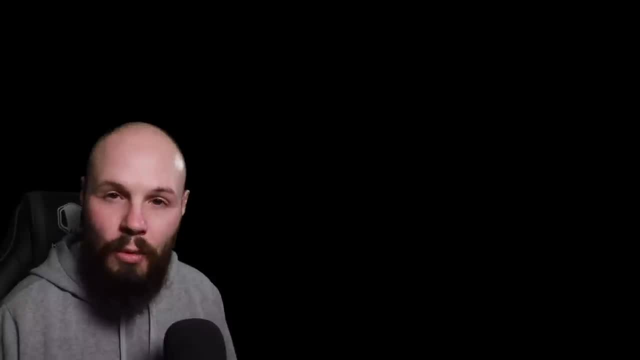 that's just one example. imagine if you're using 20 or 30 libraries. now you're probably gonna have four or five that are dealing with that and you're just- you're just gonna have a headache in your codebase all the time. so again, the rule of thumb: use them sparingly, make sure they're. 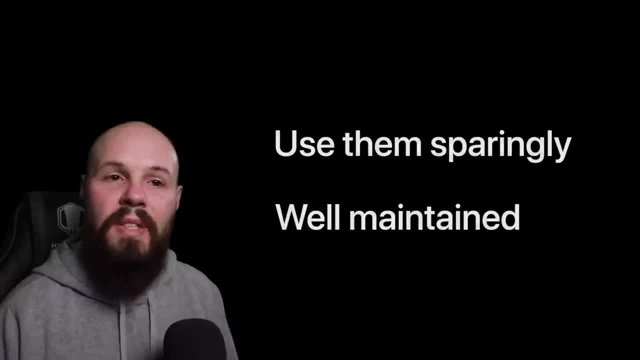 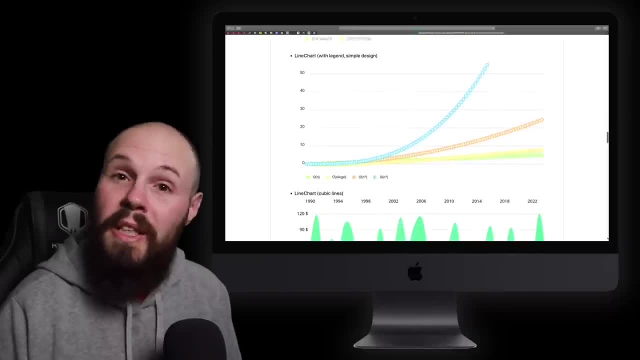 well maintained. You'll thank yourself later. Another downside to using them is you get a lot of bloat, Like let's go back to this charts repo real quick. You see all these different charts you can do like that's pretty cool, That's a pretty nice feature of the library. However, most likely if you bring in this library like we do out of Luna, 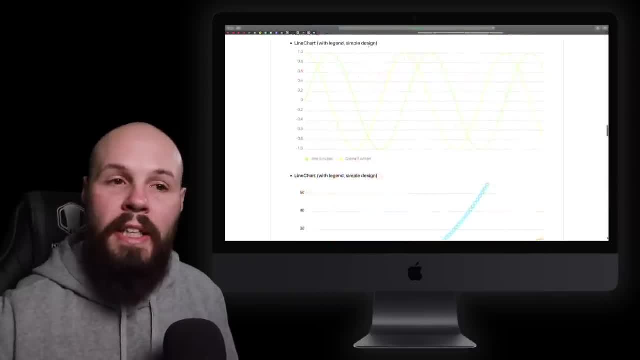 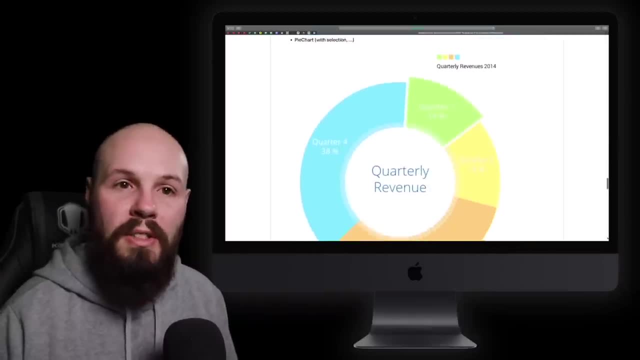 We just wanted the line chart. Well, when you bring in that library, you're bringing in all the code for all those other charts and all the functionality behind those charts. So typically, bringing in these third-party dependencies, You're bringing in a lot of bloat, meaning a lot of extra code that you don't need. 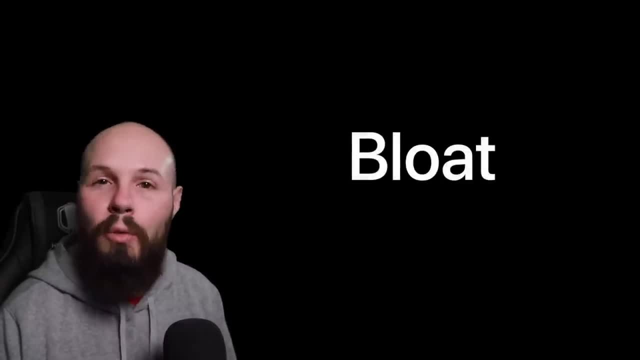 For example in the Luna codebase. I believe you can. you can run a command to see the lines of code in your project and the Luna codebase. when I did This was like six, seven thousand lines of code without libraries. when I added the libraries, Which there was about five or six of them, it went up to like sixty thousand lines. 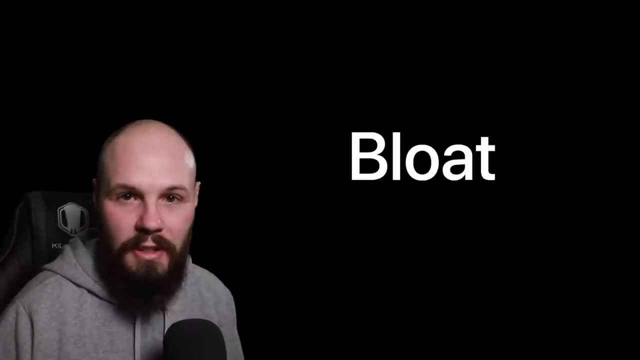 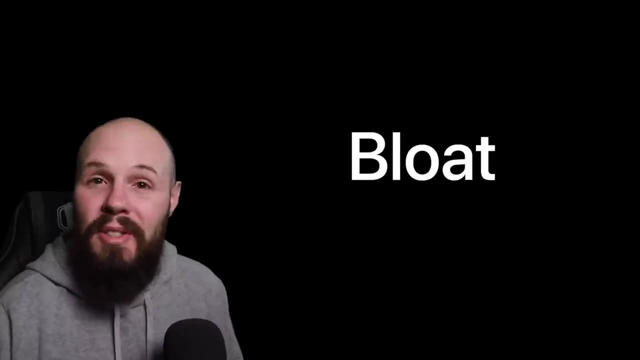 So you can see a 10x in bloat from bringing in the libraries. So just keep that in mind as well. You're really ballooning the size of your app by bringing those in, which, again, may not be a bad thing, It may be a necessity. 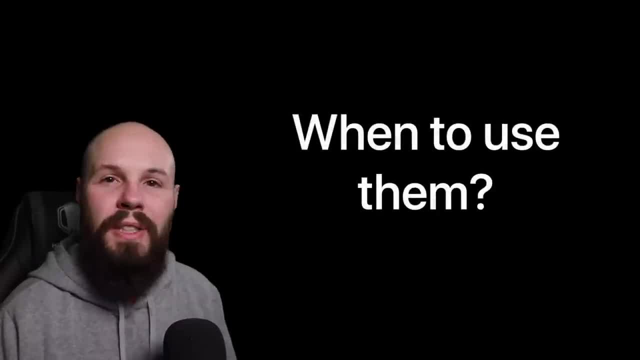 But again, just something to keep in mind. and the last bit I want to talk about is when you're deciding, Like when you should use a library, because oftentimes you know new, inexperienced developers will say: why would I reinvent the wheel, Like somebody's already written this code, Let me just use that. it'll save me two weeks worth of work. 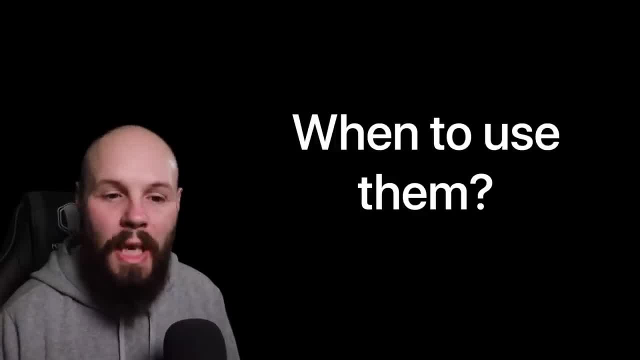 And I get that thinking. but if you're building a product or you're building a start-up or a business around your app And you plan on this app being around for two, three, four, five more years, That two weeks or a month you took up front will be nothing in the grand scheme of things and you'll be so much better. 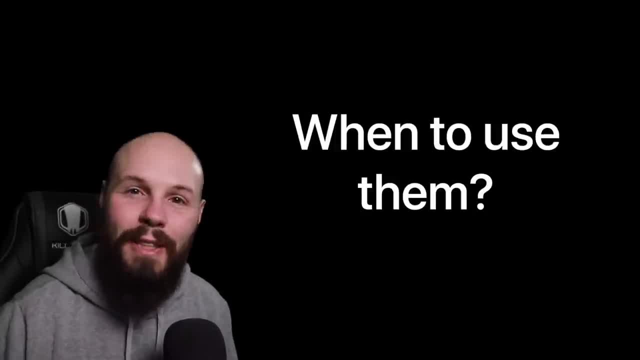 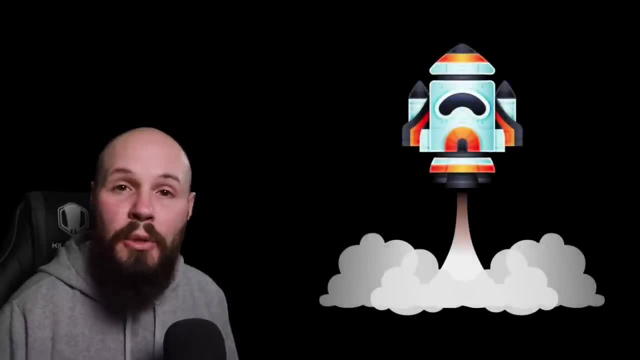 Off that. you wrote it yourself And you have control of that code. you're not depending on some library to do it. So, again, these are just some things you should be thinking about when it comes time to use a library. again, Use them sparingly if you overdo it. 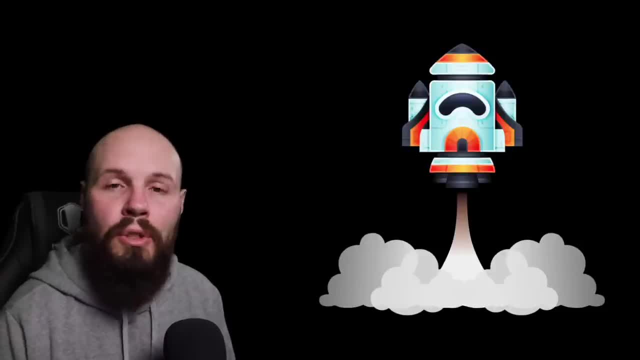 You're gonna have headaches, trust me. and then also the ones you do choose to use, make sure they're actively Maintained and they're gonna be around for the next year or two. So that's the overview on libraries. Of course, as always, if you have questions about this, read the comment section or you know. 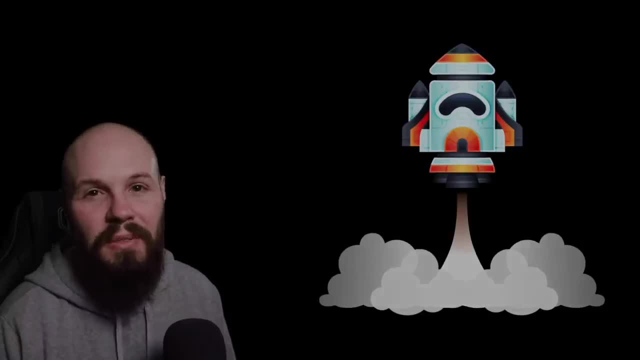 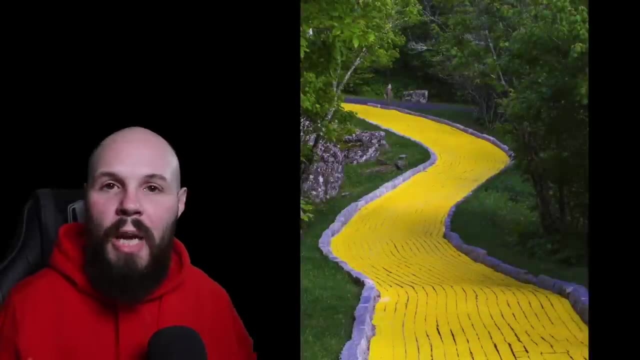 Post a comment down below and, as always, we have the slack channel. See you in the next video. You, When we're building or designing our apps, Oftentimes we start with what's called the happy path or the golden path. right, This is how. this is how we're designing our app. 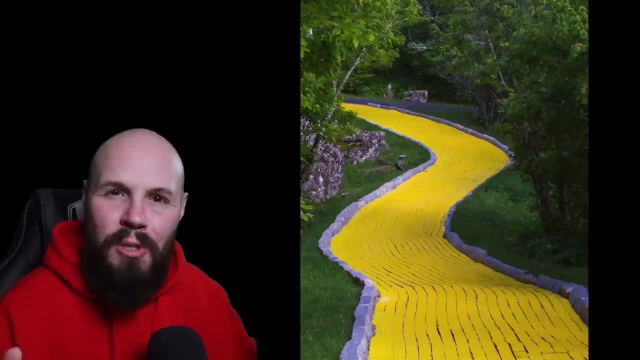 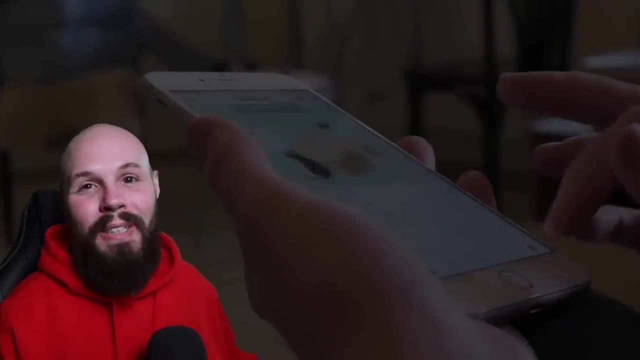 This is how we want users to use our app. This is how users are supposed to use our app, right? However, once your apps are out in the wild, out in the real world, It doesn't always work like that, and you have to handle what are called edge cases, right? 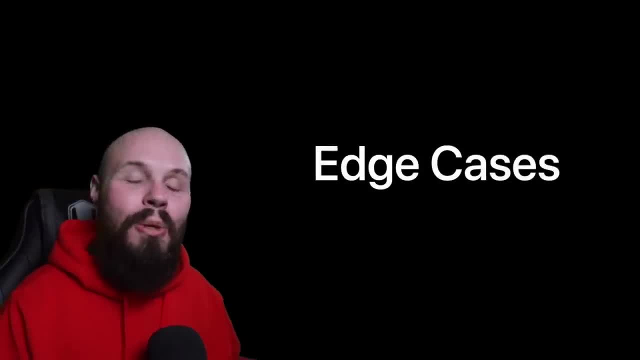 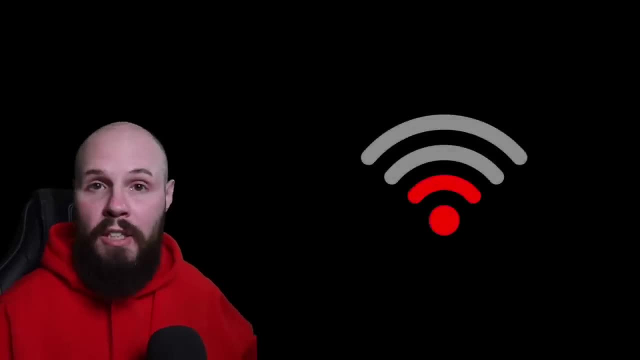 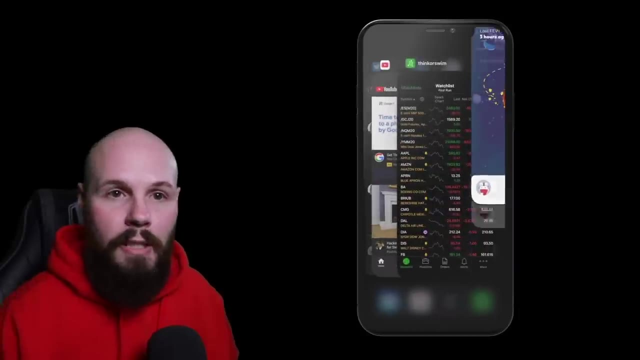 These are kind of not the normal way to use your app, but you still have to handle it. Like. let's walk through some examples. How does your app work when there's a very, very bad internet connection or no internet connection at all? Like, can you handle that? or what if you're in a really crucial function in your app and the user just kills your app right? 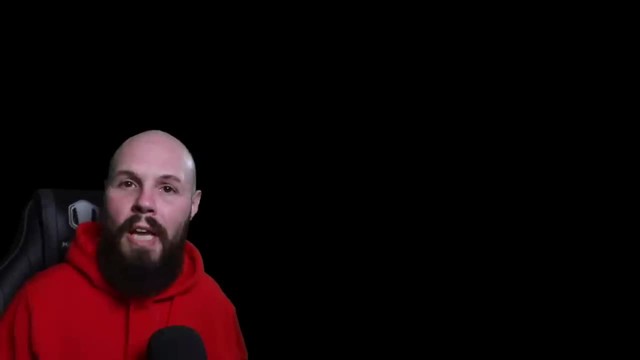 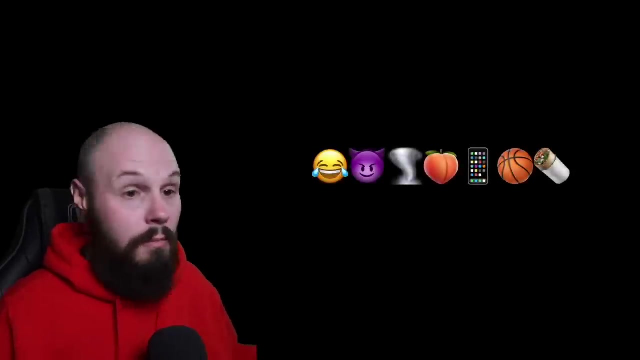 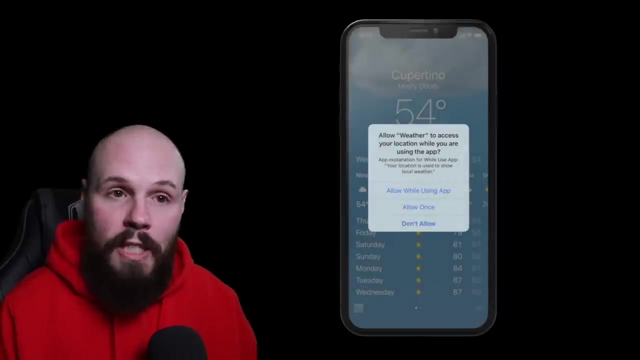 Just, you know, swipes up on the screen kills the app. How does your app handle that, or what if you're expecting an email in the field? right, You want to collect the users email and the user just types 13 emojis? Can you handle that? or what? if you know your app requires location permissions and the user actually gave you those location permissions? 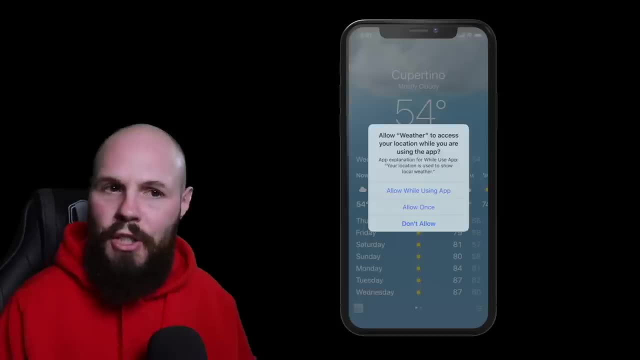 However, three weeks later they revoked those permissions. is your app able to handle that change in permissions Or will it just crash and break everywhere because you just assume that once you've got permission You would always have permission and you could go on and on and on thinking of all the crazy edge cases and handling them? 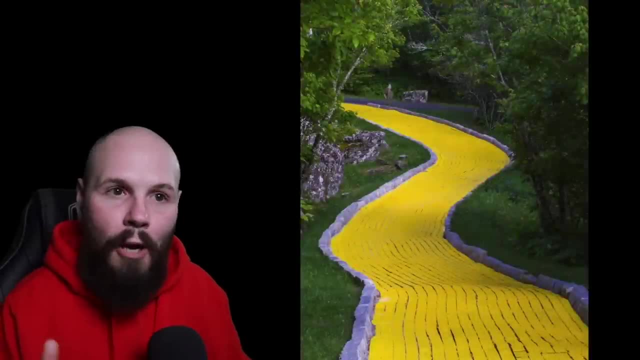 But again back to that building that happy path of the golden path of how your users are supposed to use your app. That is like half the battle right, once you get that happy path done. now you got to handle the edge cases right because, again, if you've ever built an app and handed 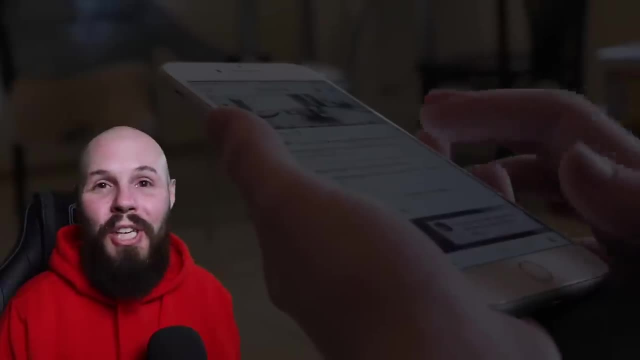 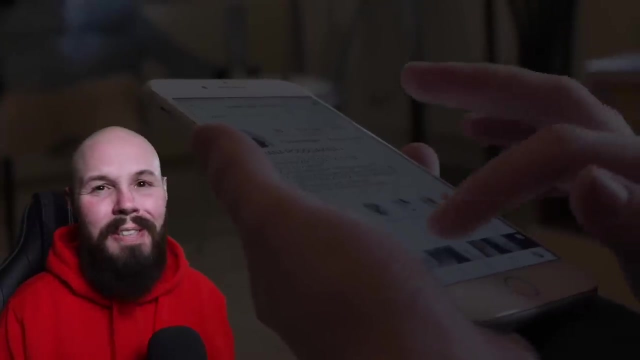 It to user and watch them use it. There's a very good chance that they are not going to use it Anywhere near the way you want them to use it or, like I said, how they're supposed to use it. Let's finish off the examples with one more that's actually very common and that is handling empty arrays right. 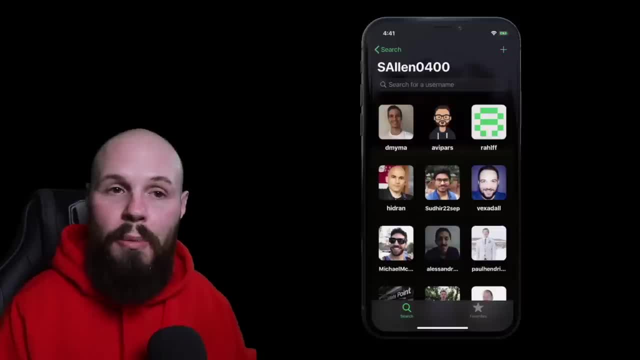 So, for example, let's say we're showing a list of followers on the screen that we got. Well, the happy path is to always expect, hey, there's gonna be followers. Well, what if that array is empty? What if the user has no followers? Are you just showing a blank screen? 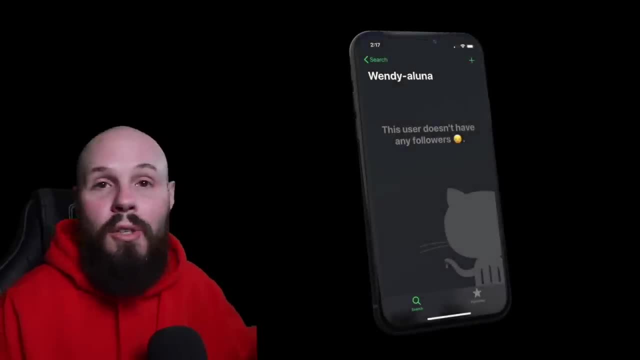 Well, you shouldn't. you should show an empty screen State saying, hey, this user has no followers, right? So even though an edge case may not crash your app, it may lead to a poor user experience, right? Have you ever used an app just came to a blank screen or the app just froze and did nothing at all without telling you? 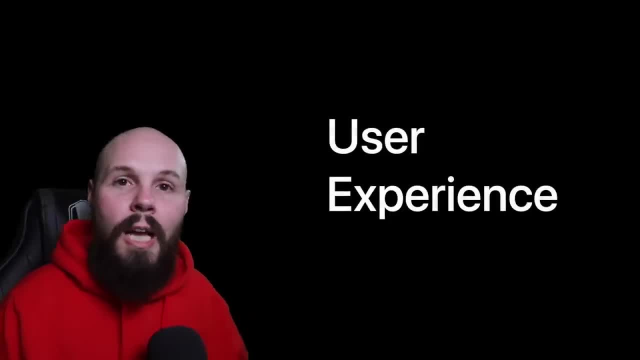 Anything right, like the bad user experience. So oftentimes, handling all these edge cases is more about creating a smooth user experience as the user uses your app. Quote-unquote: improperly right. We call it fail gracefully right. It's impossible to build an app that doesn't. 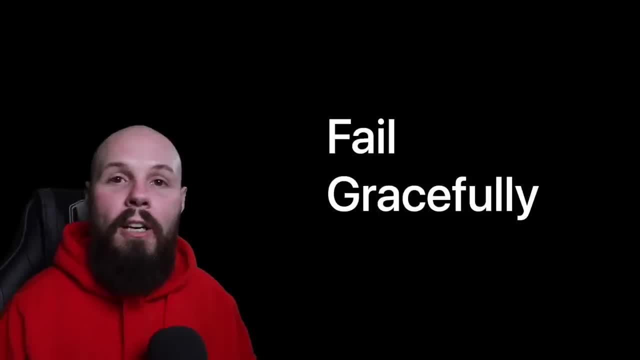 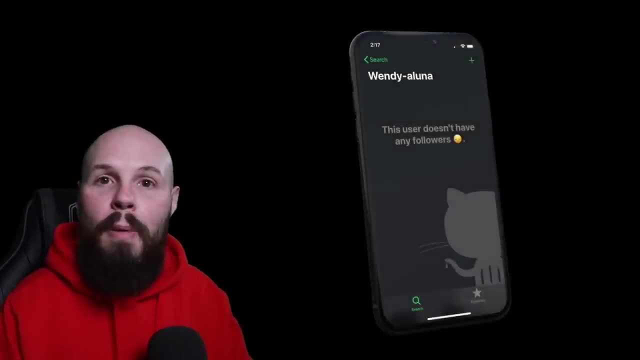 Fail or doesn't have a situation where it can break. the key here is to fail gracefully in that like, okay, something bad happened, now Let's handle it Right. give the user an informative error message So they know what's going on and move on right. 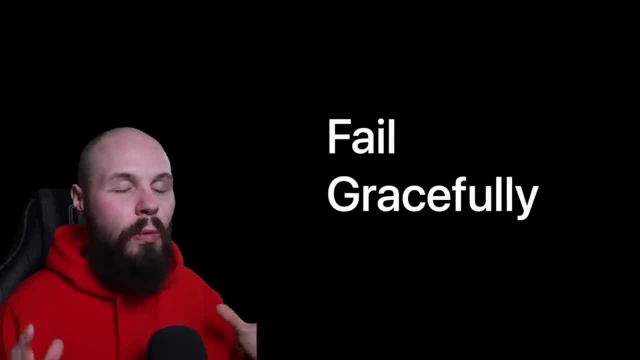 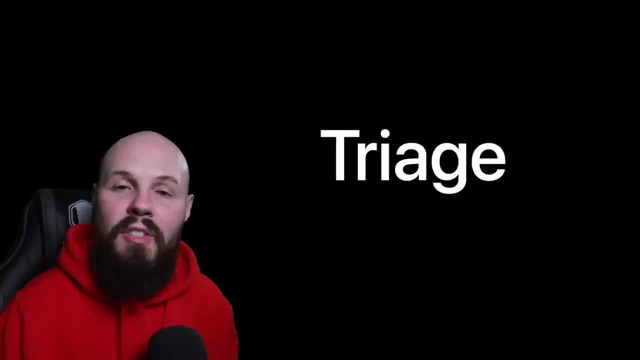 That's called failing. gracefully Now, as I mentioned a little earlier, like you can get real crazy thinking of edge cases, But this is where your your triage skills come into play, right? You don't have to fix every single edge case, right? Because if, if there's an edge case that's so crazy and wild that it only affects, you know, Zero point one percent of your users, like maybe you can spend your resources in your development time on other things rather than fixing all those Super crazy zero point one percent edge cases right now, if something affects two to five percent of your users. 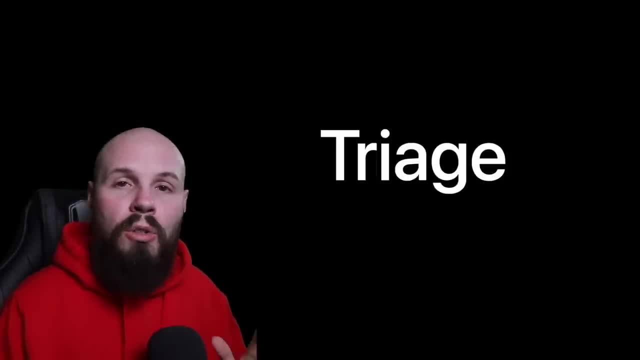 Of course you want to fix that like right away, and also your size matters, right? So I just said zero point one percent of your users. Well, if you have ten hundred thousand users, sure That's not a large number. if your Facebook zero point one percent of your users is, 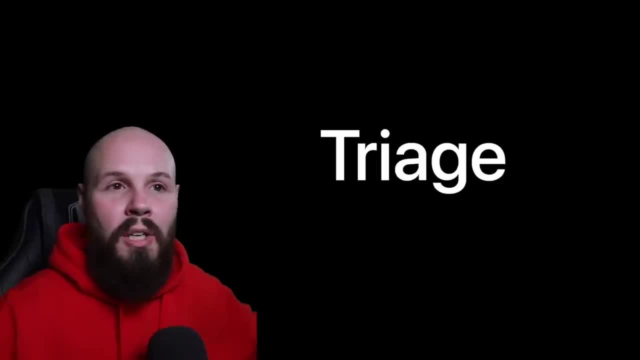 A very large number. So, again, the larger your user base, the more you have to fix those crazy corner cases because, again, that's a lot of people out there. But, like I said, what edge cases you actually go fix is a decision You have to make, one based on your resources, like: how much development time do you have? 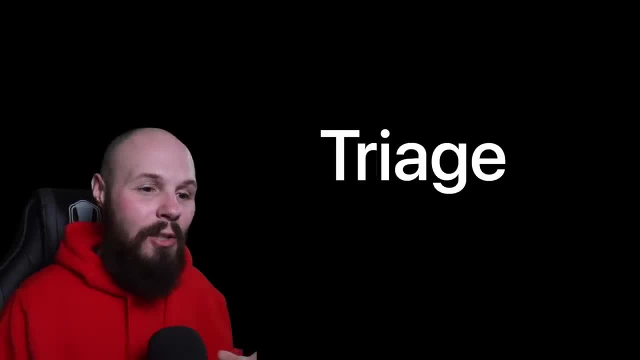 How many users is it affecting, like what percentage? so all that comes into play when choosing Which ones to fix in, which ones to just live with right, and that's what's called triage. So thinking of these edge cases not only makes a great product, But it's going to help. 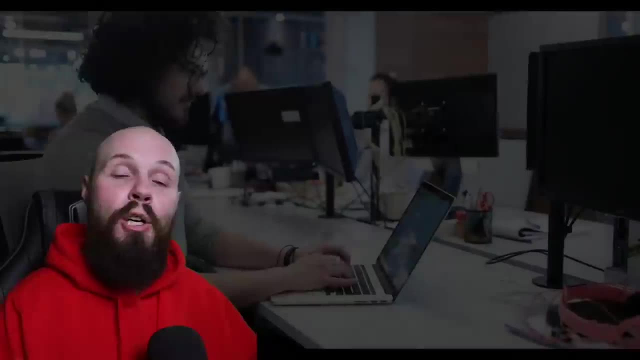 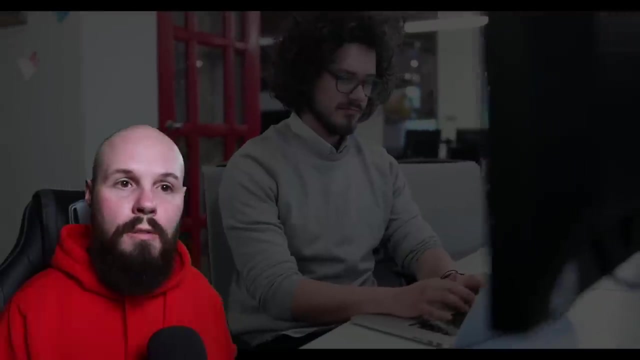 You in job interviews as well. often for a job interview You'll get a take-home project to do, or maybe you're live coding on a whiteboard, or you know You're on a phone screen where you have to do an hour coding on a computer. You should absolutely be thinking and telling your interviewer like okay. 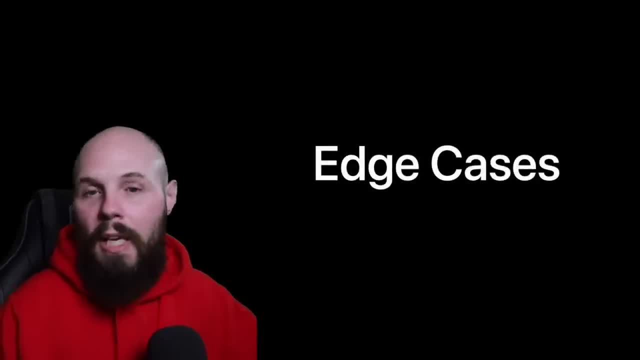 This is a potential edge case, or this is how I would handle the array being empty. Thinking of those edge cases is absolutely vital in those interviews because again, it shows that you're an experienced developer Who will think of those things. Oftentimes it's the very beginner developer that doesn't think of the crazy edge cases. 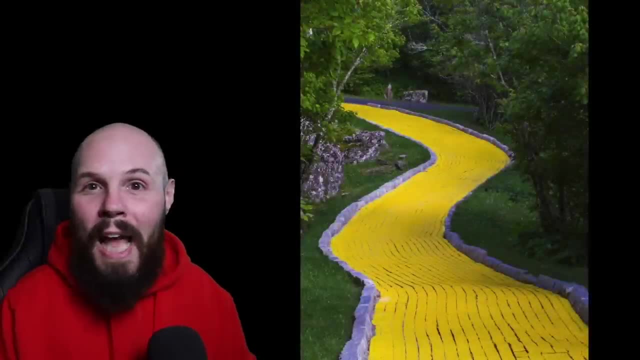 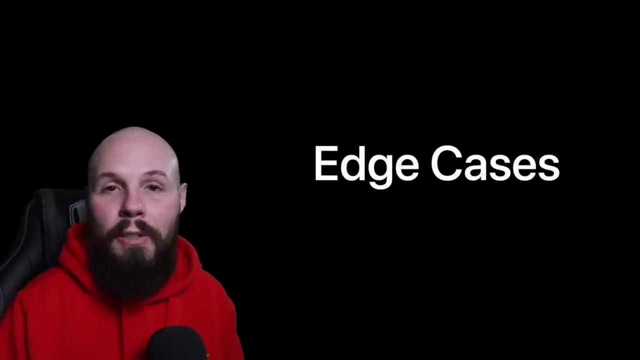 And they only handle the happy path. and then when a user veers off that happy path, You know things go crazy. so, again, the edge cases can help you make a great product as well as help you in interviews. There's a high-level overview of edge cases. I think this could be fun. 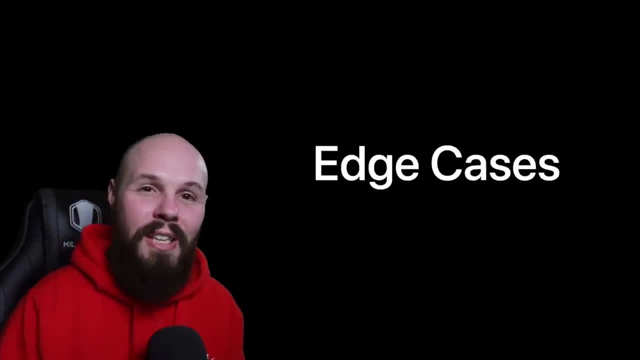 Feel free to leave some crazy edge cases you've come across in the comments or in the slack channel. I think it would be kind of fun to just share some weird ways users used your app that led to a crazy edge Case that you had to fix and I think you know the community at large can benefit from that knowledge as well. 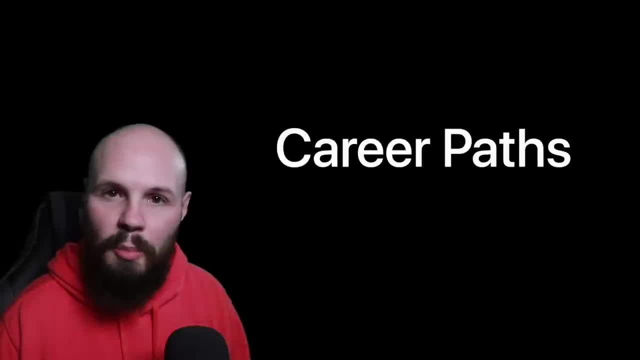 I'll be doing a video on that in a couple weeks. Being a software developer- you know, not just an iOS engineer, But just any general software developer- is probably one of the most flexible Careers like a person can have, and that's why I love it. 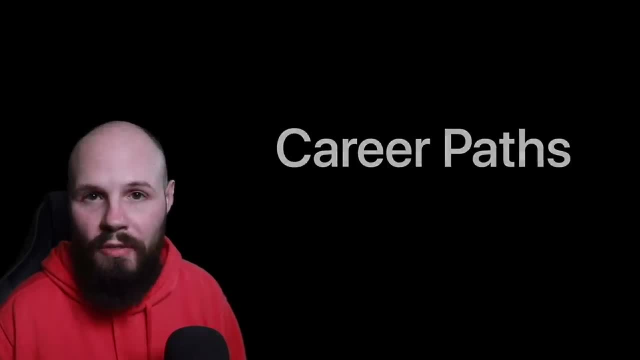 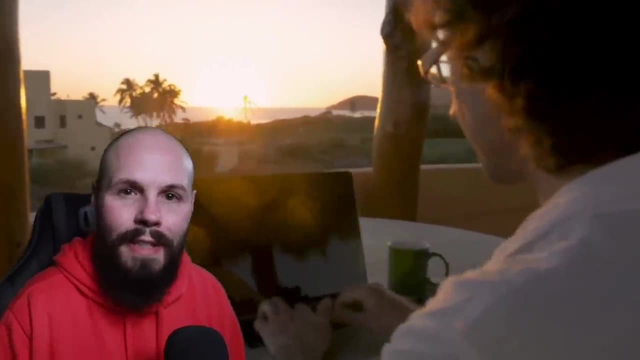 You just you have so many options, and that's what we're gonna talk about in this video. right, You can go the big company route. you can go the small startup route. You can go independent contractor or freelancer, where you're like a digital nomad. 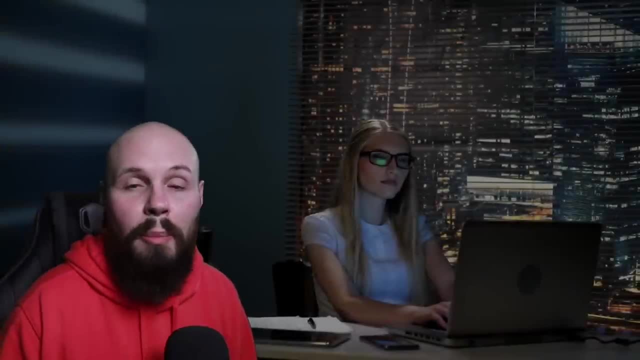 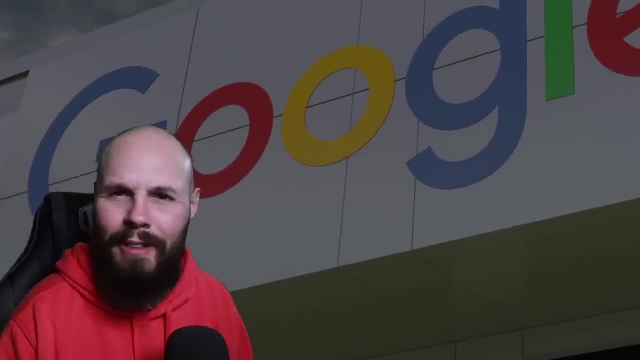 You can work from anywhere. you can build your own products, build your own companies, like the options are almost endless. so let's talk about Those main ones first up. let's talk about the path of going to a big company like we're like an Apple, Google. Let's get the obvious stuff out of the way first. right, Like, the pay is gonna be very good. 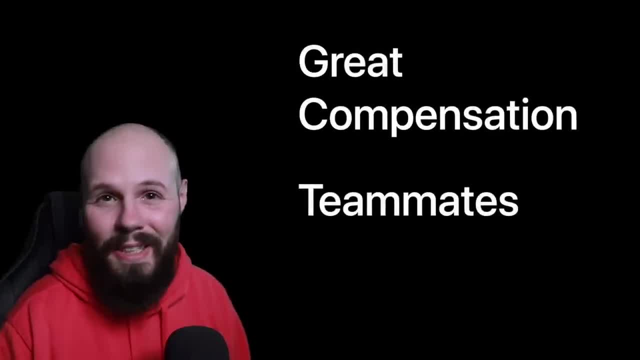 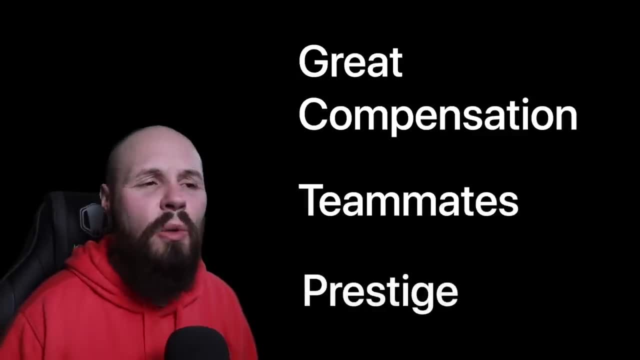 You're gonna have awesome health benefits. You're gonna work on a great team. You're gonna have the prestige of that name on your resume, which is going to help you. You know the rest of your career. so a lot of good stuff and going to a big company. 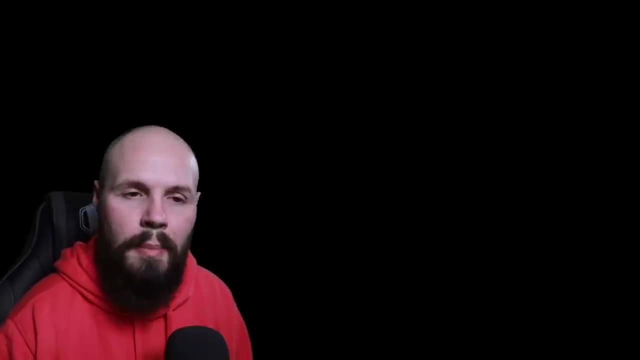 Um, there are some downsides. oftentimes- not not every time, but often- you will end up specializing in one area, Like the kind of the joke you know. the exaggeration is like: oh, you'll be The login screen person and that's it. And again, that's not always the case, but you tend to have narrow 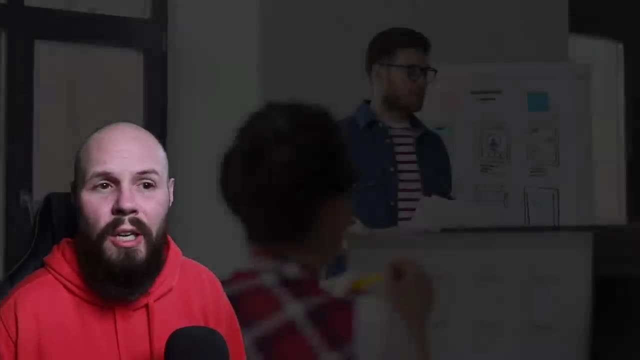 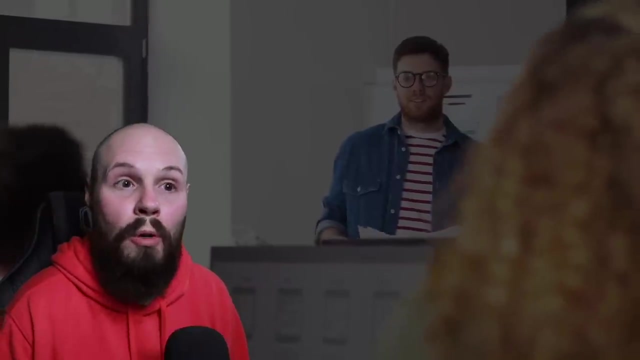 Responsibilities. at a big company- right- you specialize, whereas at a start-up, you have to wear a lot of different hats. right- Even though you're a developer, you may be getting into marketing or or product and all this stuff. right, You have to do a lot more because there's only, you know, a small number of you. 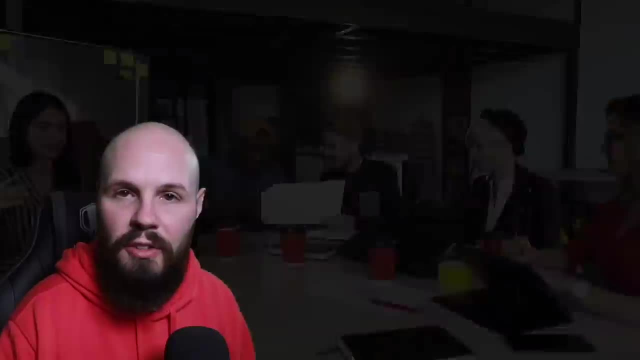 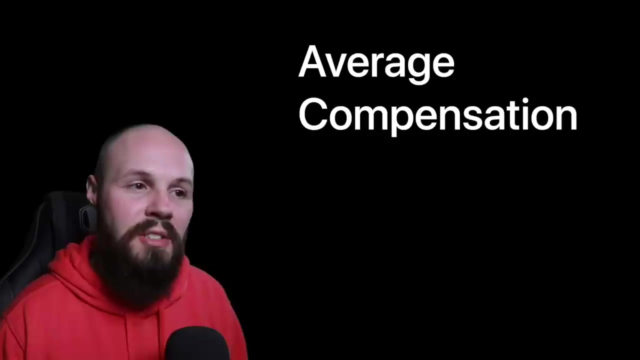 So now let's talk about those small startups, right, They? they tend to have benefits as well. Now, if it's a super small startup, you may not have benefits, But you know, I would say anything: five employees and above, you're probably gonna have benefits. 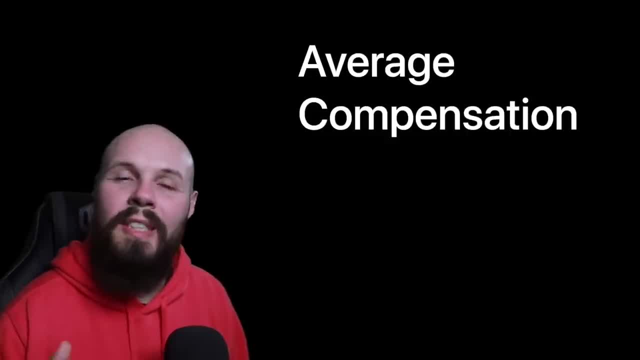 But the pay is probably average. oftentimes startups can't compete with those big Google, Apple pay. But the trade-off you get at a start-up is you often get equity in the company. right, You get some shares. you know If the company were ever to get acquired or go public, those shares would theoretically be worth a lot of money if you got in. 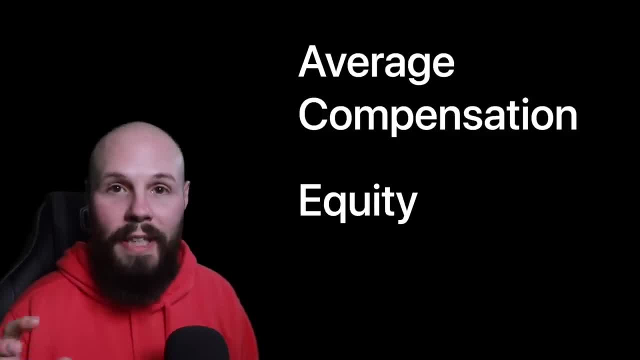 Early enough. now here's the thing for every they call it an exit. for every good exit, again, That's when a company gets acquired or goes public. You know, for every good exit There's a hundred where those startups fail or go out of business Or those shares end up being worthless. so even though getting equity in a company is cool, 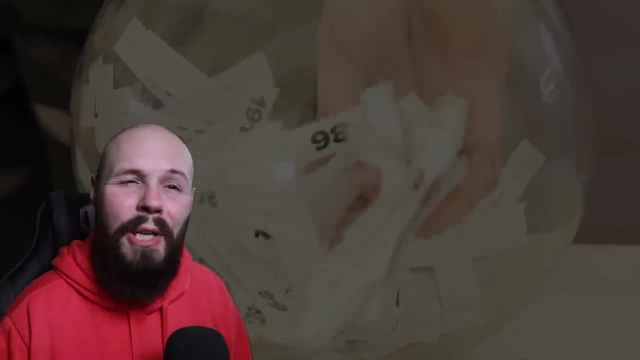 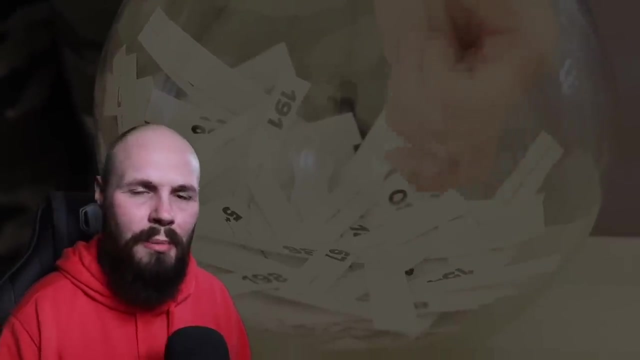 I consider them to be almost like lottery tickets. right, I don't value them too much because the the odds of them hitting are pretty slim. and not only are the odds of them hitting Pretty slim, but you also have to be at that company for like four or five years. 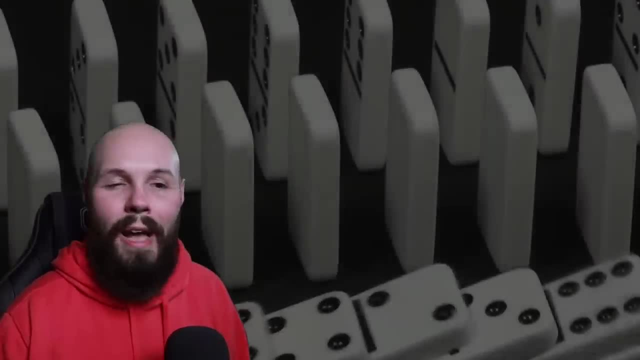 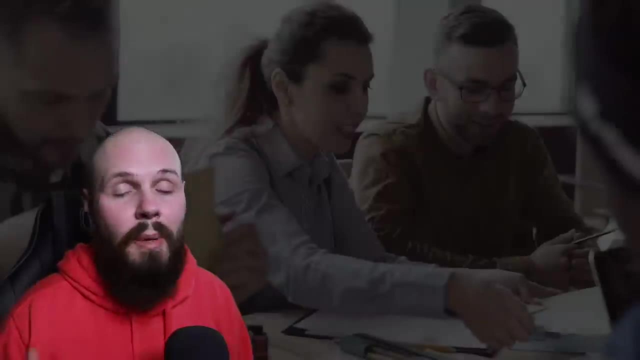 Which, again, nowadays many people don't stay at a company for that long. So a lot, of, a lot of dominoes have to fall into place for that to work out for you. But I actually prefer small startups to big companies. It's my personal preference, right? because I like the 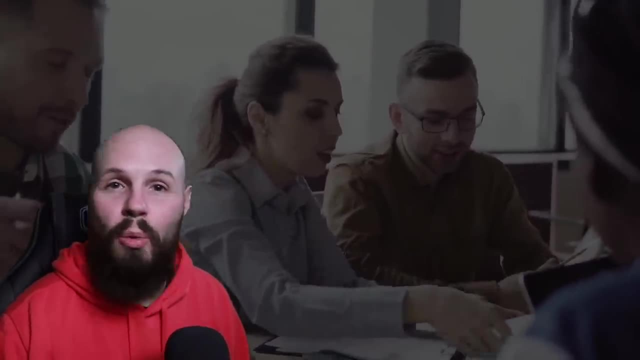 Tight-knit team again. I've worked at companies, you know, five people to 25 people and everywhere in that range, And that's just pretty cool, right It's. it's a tight-knit team and I like wearing many hats, right. 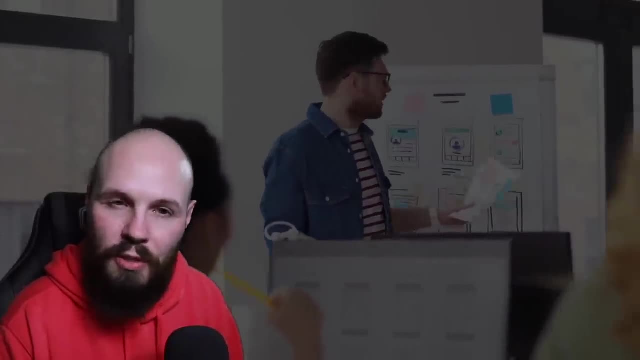 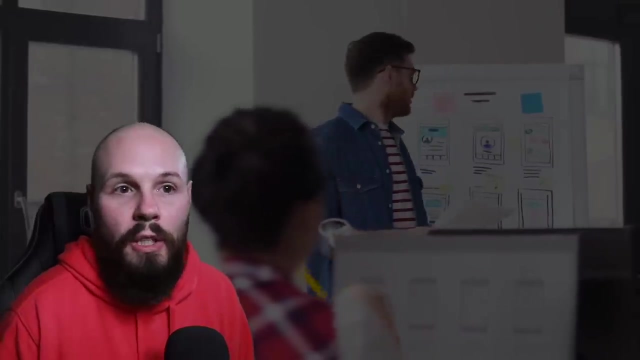 I don't think I would enjoy being a specialist and only programming and working on this one thing. Like I enjoy being part of the marketing discussions at the startup. I enjoy having input on the product. I enjoy, you know, helping hire a marketing director, right. Like I like having my hands in things. 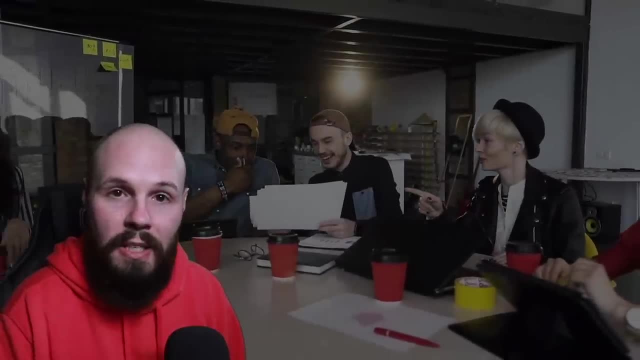 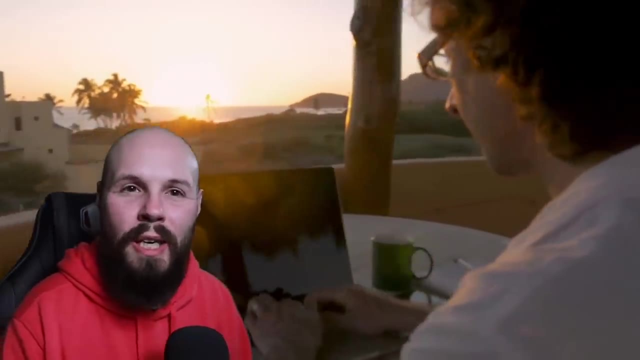 I don't know, I just find it interesting. That's a personal preference. You may like specializing, but I just wanted to Tell you the difference between going to a big company and a startup. now let's talk about freelancing, sometimes also called independent contracting. 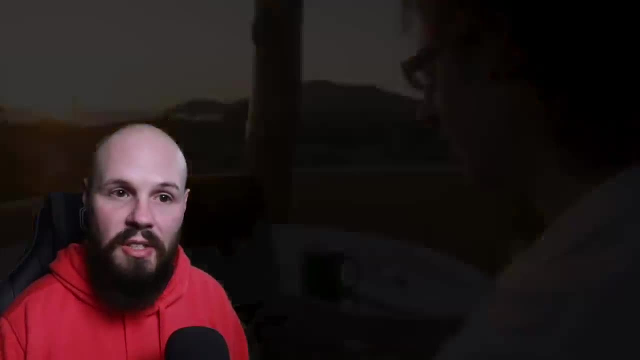 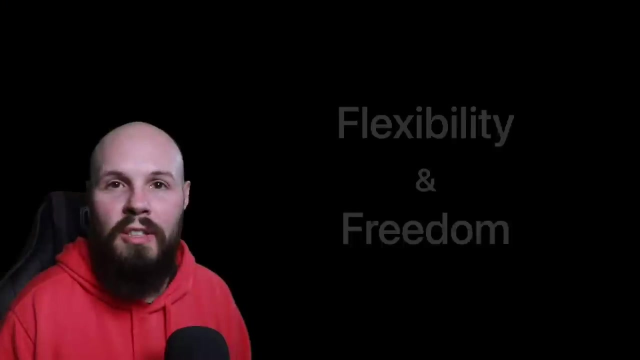 But the idea here is that you're working on a contract basis on you know a couple different apps. Maybe you have one contract as a big one, Maybe you have a couple small ones, but the benefits here is just flexibility and freedom. You get to kind of you work remotely, right. 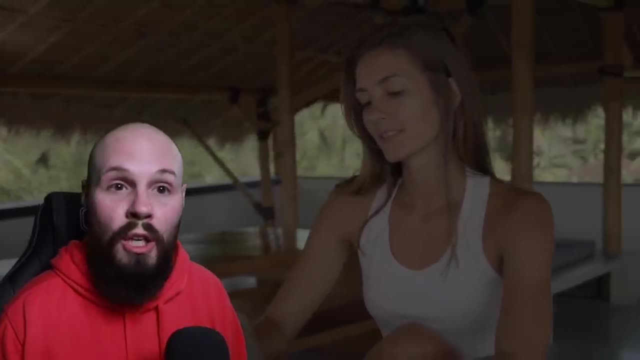 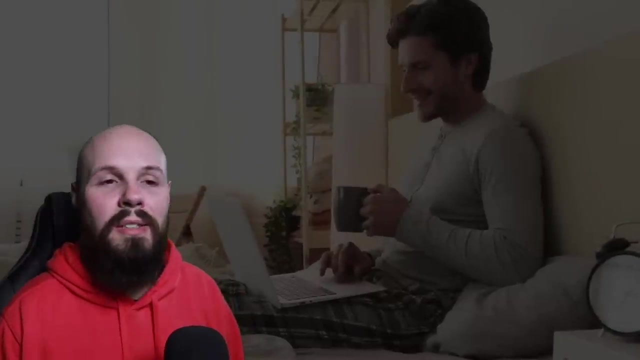 You heard the concept of a digital nomad, where people just travel the world Working remotely on contracts out of coffee shops like that sounds like a pretty fun life. or you can just work from home. That works too. but the reason people like This is because there's no commute. they make their own schedule. 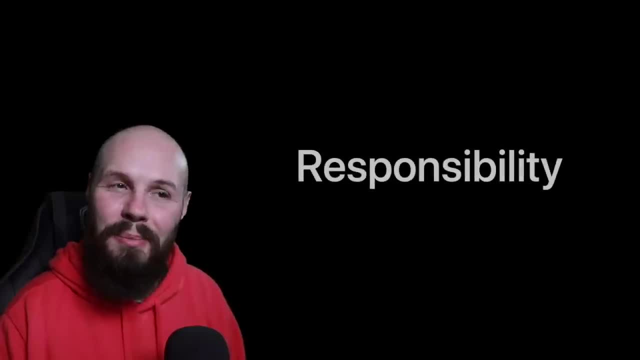 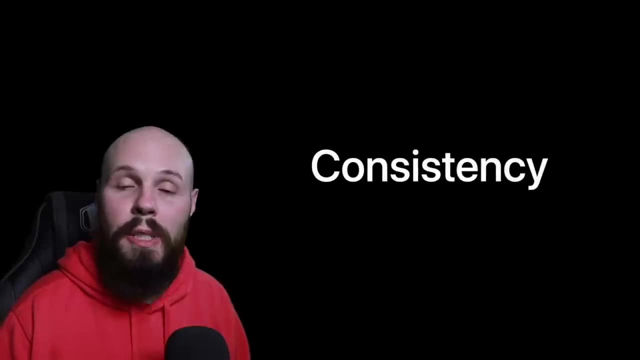 You have a lot of freedom, but with a lot of freedom comes some downside and responsibility. So contracting is great, But the hardest part about it is getting a consistent stream of contracts right, Because if your contracts are up, you're not getting paid. you go on vacation, You're not getting paid. 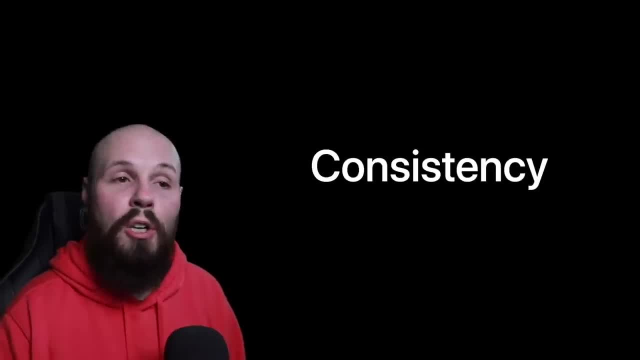 It's. it's just a different lifestyle. For example, when I was contracting earlier in my career, I had another contract lined up but it wasn't starting for four weeks, So I couldn't really like line anything up to fit in that Four weeks, so I just went without getting paid for four weeks, and that's not uncommon for contractors. 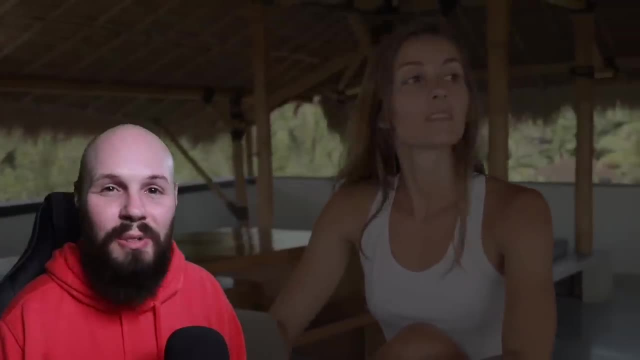 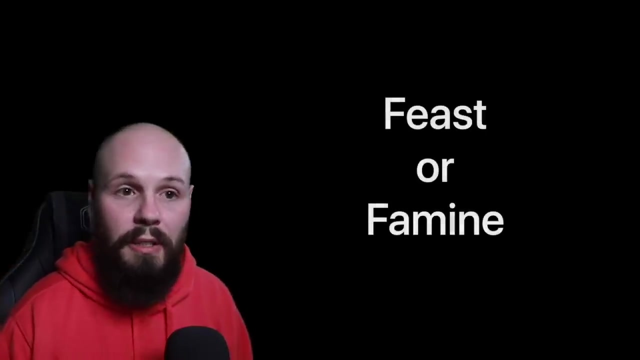 So if you like that freelancing lifestyle, that sounds awesome traveling the world. I know it does, but it's it's hard. not gonna lie, It's hard and my recommendation- because they call it feast or famine: You'll have some periods of time where you're making so much money. 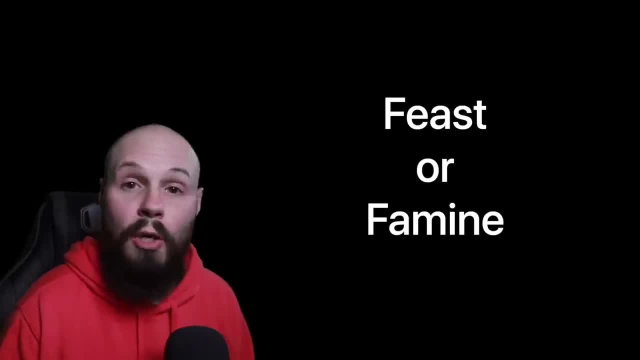 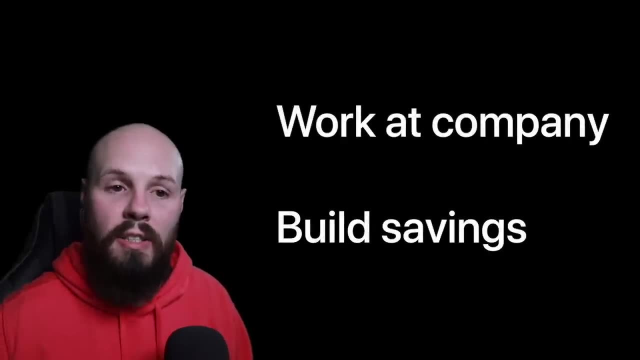 And then you have other periods of times where, like, you can't find a contract and you're making no money. So the recommendation is, if you want to try that freelancing, I would recommend working at a company first, knowing you have a plan to freelance and start building up some savings. 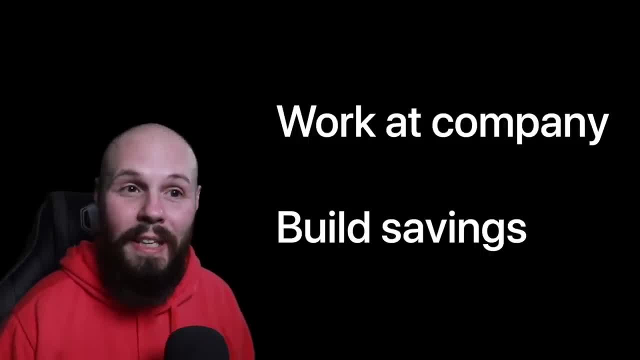 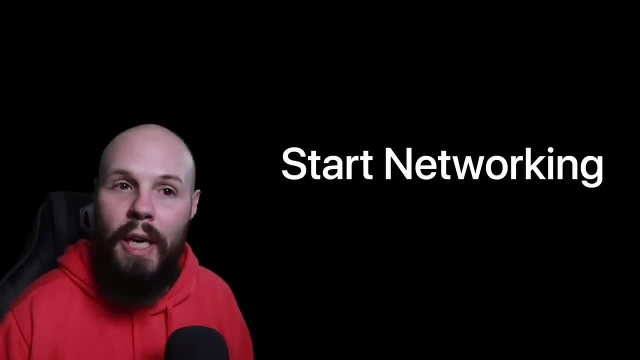 Right, because you need like an emergency fund if you're gonna be a contractor And then also while you're working full-time, you can maybe start lining up contracts on the side, Maybe. but start building connections, because in contracting your network is extremely valuable, Like that's how I get all my contracts right- my personal and professional network, word-of-mouth, the YouTube channel helps. 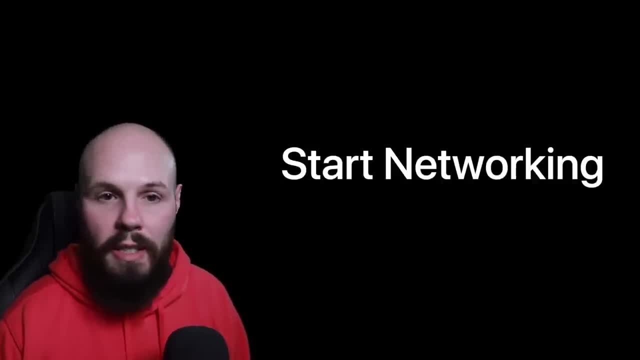 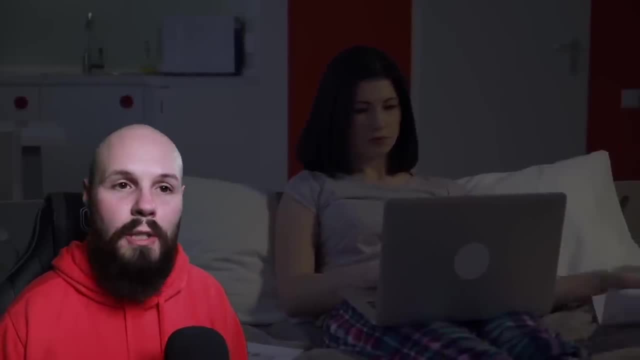 But it's never going to like up work or some internet site and finding contracts. So again, if you're thinking about freelancing work at a company, start building up your network. Maybe find a small contract or two, Build up a nest egg of money and then make the leap. trust me. 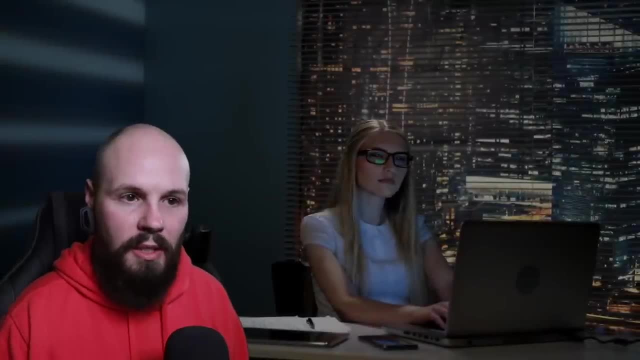 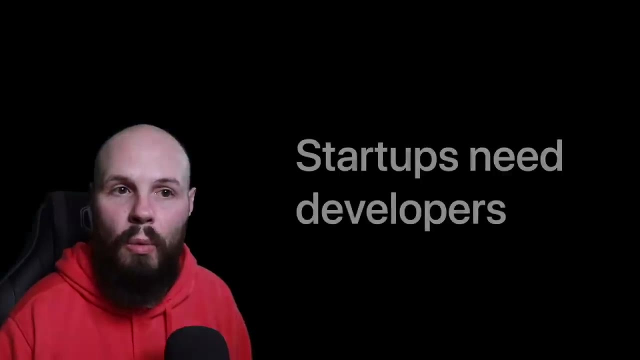 You'll thank me for that advice later. Now let's talking about building your own thing, because this is kind of the most vague or the most flexible, But it's great if you're entrepreneurial and you want to, you know, create your own startup. One of the biggest problems startups have is finding technical people, finding developers that are good. 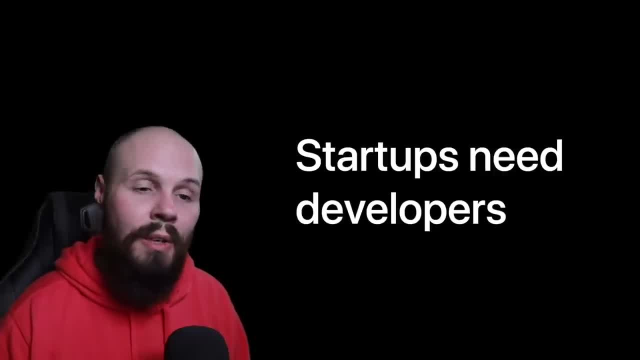 So if you can just eliminate that problem by you being the developer, you have so much freedom And again like: if you have an idea, build it, like it's almost like a superpower being a developer. right, You don't even have to go as far as like building your own startups. 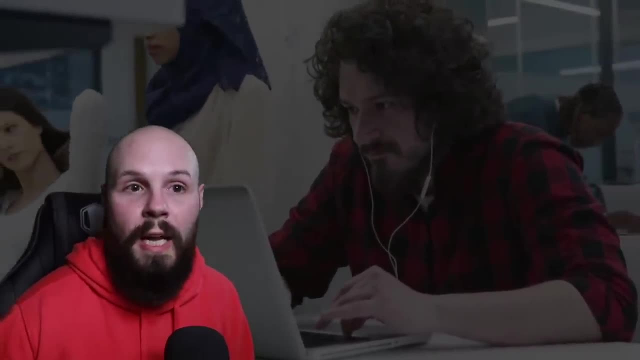 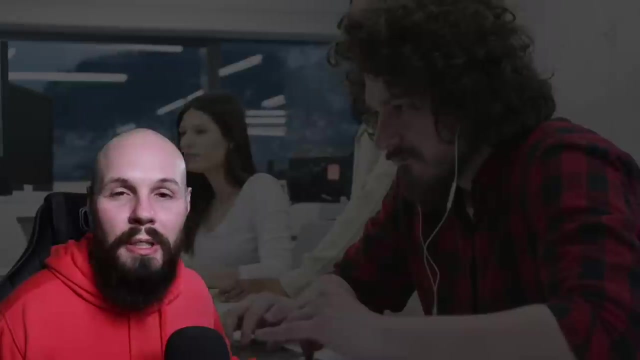 Maybe you can just build your own portfolio of independent apps and then, over time, those ten apps are making enough money for your living. Right, It's just again. This career path is is so flexible: big company, startup, freelancing, building your own thing. I just love it. 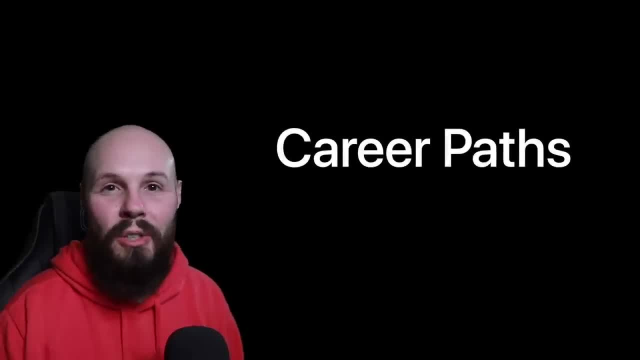 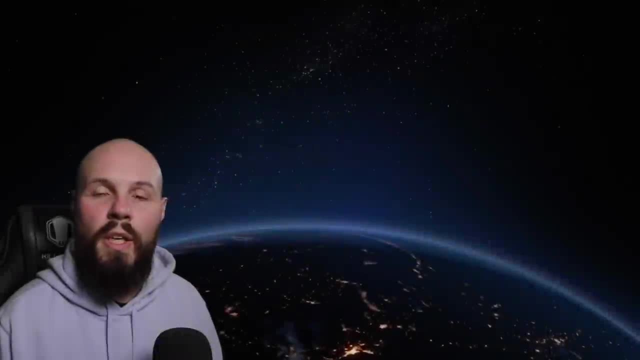 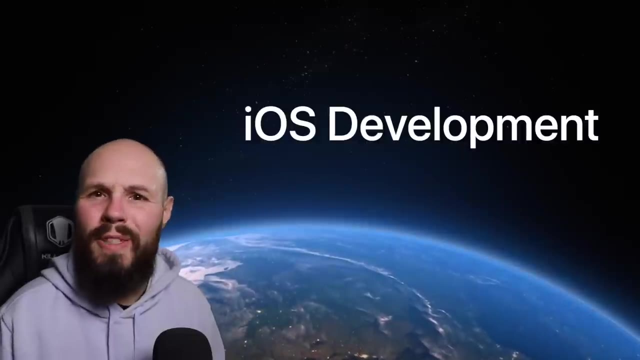 I'm so happy you're on this path and I hope that I can help you get your start, because it's a it's a wonderful life. I'm not gonna lie. In this section, we're gonna talk about the world of iOS development, Some of the resources that I use this day to continue my learning, and then some of the resources I use back when I first got my start. 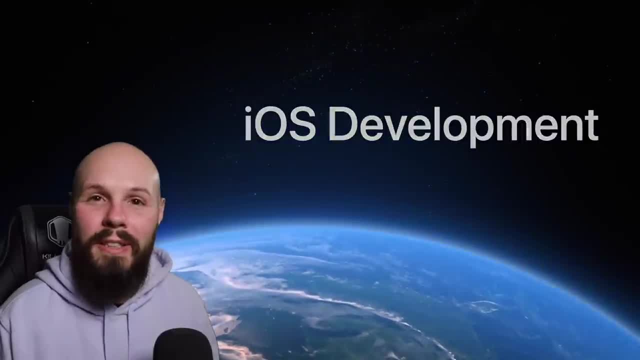 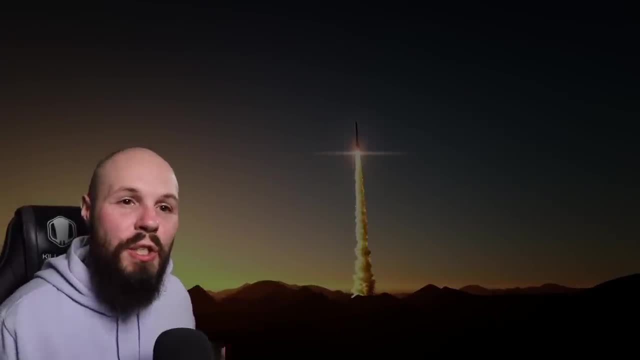 Now, I know this section isn't teaching you how to code directly, But in my opinion, it is still insanely valuable because, again, the whole point of this course was to set you up for success. right, I want you to use this foundation to continue your journey, continue building upon it towards a successful career. 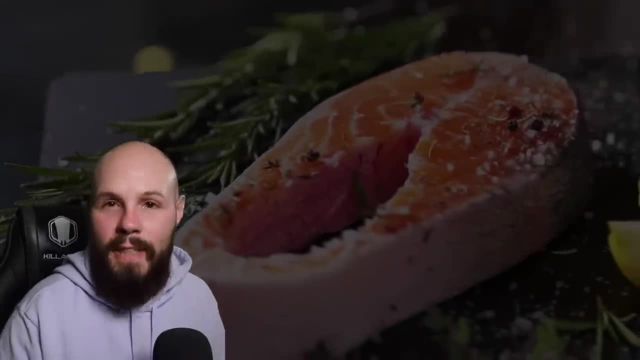 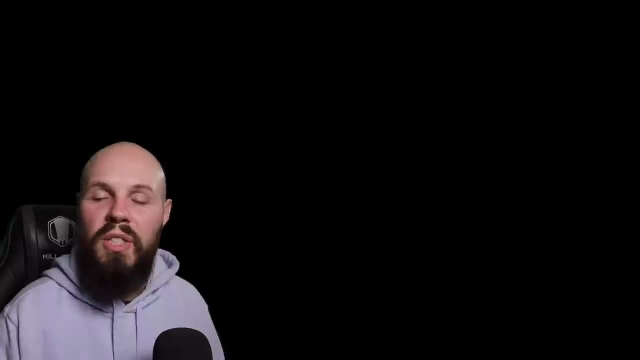 You've probably heard the phrase. you know: give somebody a fish and they eat for a day. teach somebody how to fish and they eat for a lifetime. Well, I'm trying to teach you how to fish, And that's what this section does. we'll cover a bunch of different blogs and website that I visit on a regular basis. to keep 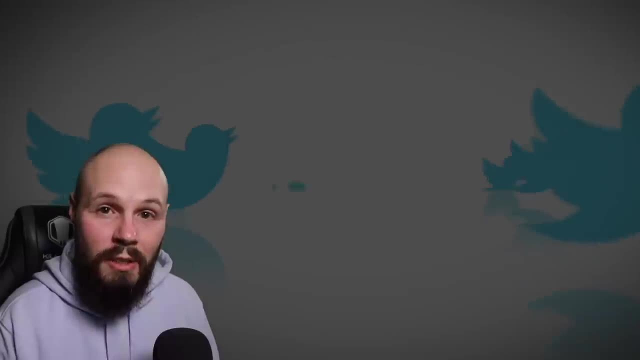 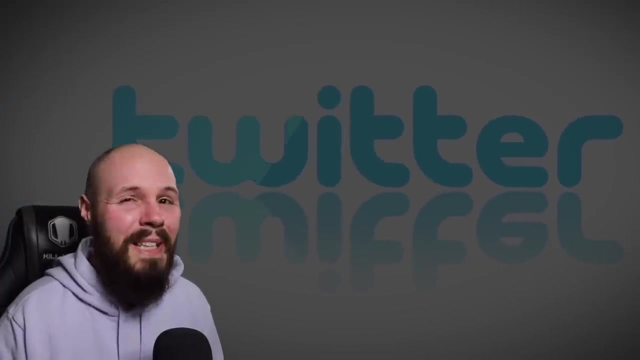 My knowledge up to date, I'll show you how to use Twitter most effectively. Yeah, I said Twitter, believe it or not. as a developer, Twitter Might be the most valuable tool you have when it comes to learning and networking, getting jobs, getting that interview Like Twitter is insanely powerful and I know what kind of gets a bad rap. all the political and bullying stuff. 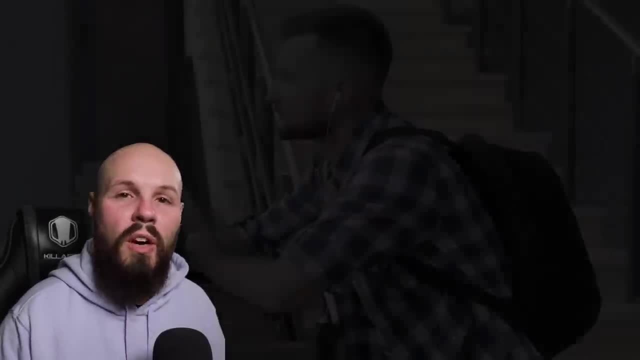 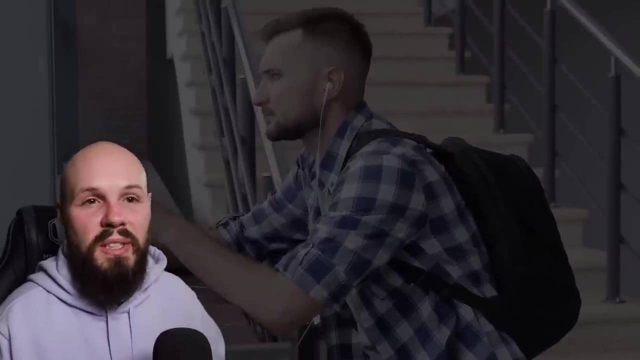 But developer Twitter is amazing and we'll also cover a bunch of Recommended books, recommended podcasts You should be listening to, because I believe in complete immersion when you're learning this stuff, and the more you immerse yourself in this world, The better you're going to learn it and the faster you're going to learn it. and then we'll also talk about 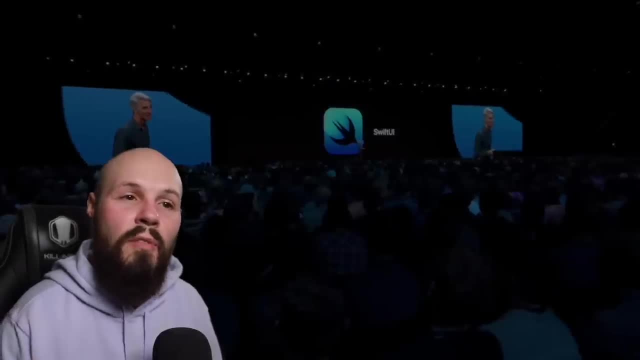 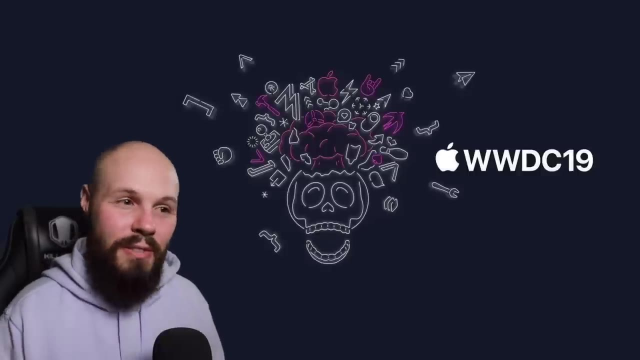 WWDC and what that is. if you're not familiar, that's the worldwide developers conference that Apple puts on every year in June, and We'll talk about why it's the best time of year for iOS developers. It's like Christmas, and if you don't celebrate Christmas, whatever happy time of the year you celebrate, It's better than that. 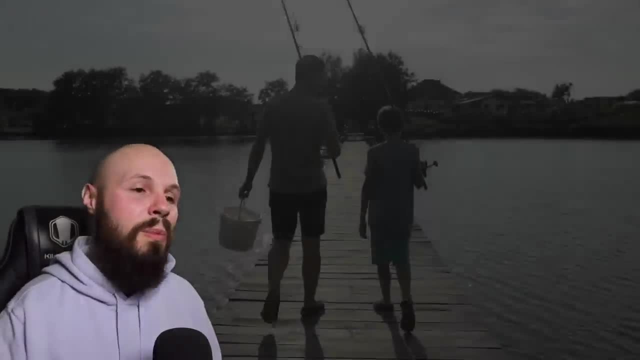 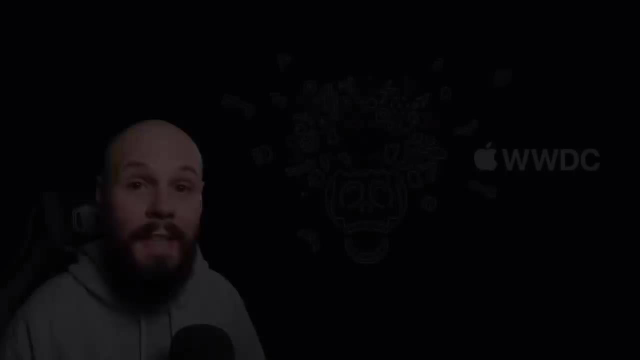 For iOS developers, and we'll talk about all that. so onward with this valuable section And I hope by the end of it you at least know how to fish a little bit. Let's talk about my favorite time of year. like, I literally take the week off of work for it, and that is. 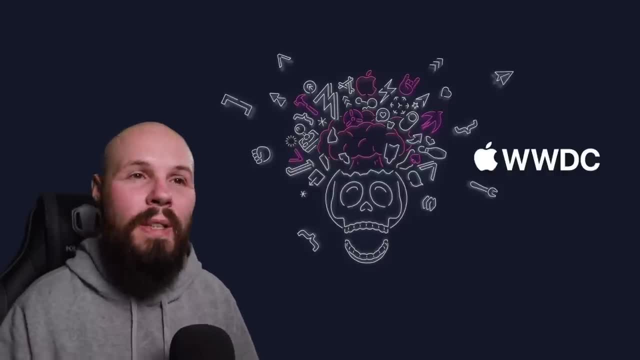 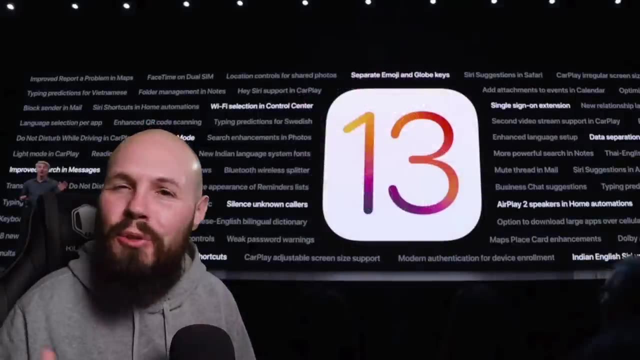 WWDC, which stands for worldwide developers conference, and what that is. that is Apple's big conference that they put on every year, Usually the first week of June, where they announce all the new stuff, the new toys for developers. right, This is where you get your first. 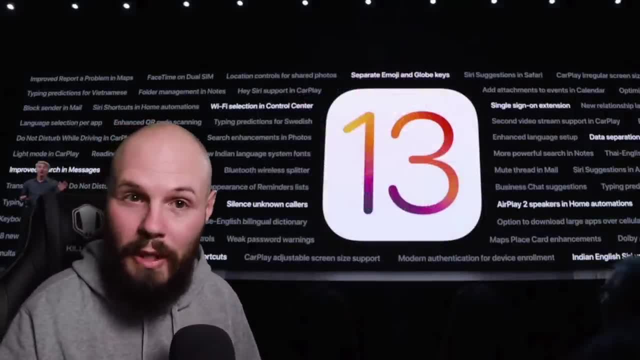 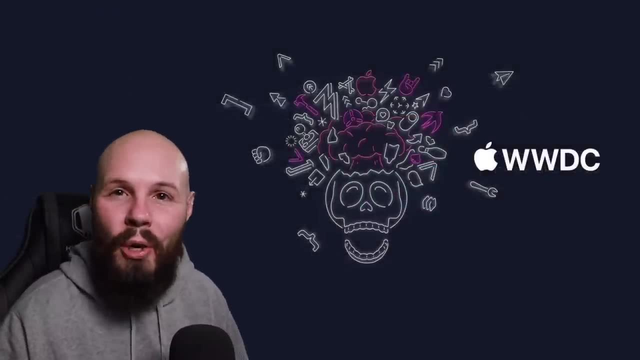 Sneak peek at the new iOS right like coming up in 2020. It'll be iOS 14, all the new stuff in Mac OS, Etc. as developers, you'll be able to download the beta to put it on your phone to play with all the new stuff. 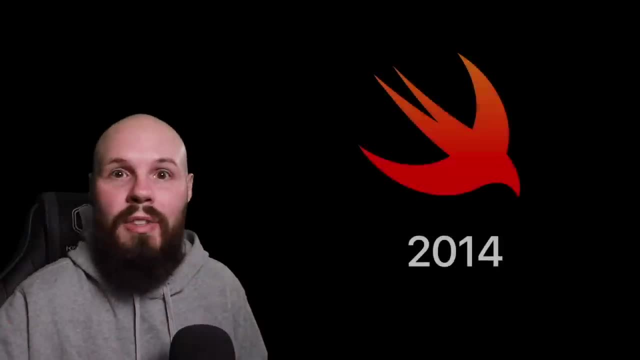 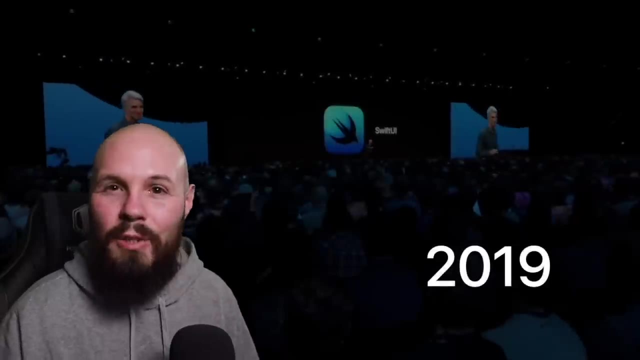 You'll see all the new frameworks coming out, Like, for example, Swift itself was announced- a surprise announcement, you know, at WWDC back in 2014- Swift UI surprise announcement 2019 WWDC. So this is when all the big stuff happens. It's the best time of year for iOS developers now. 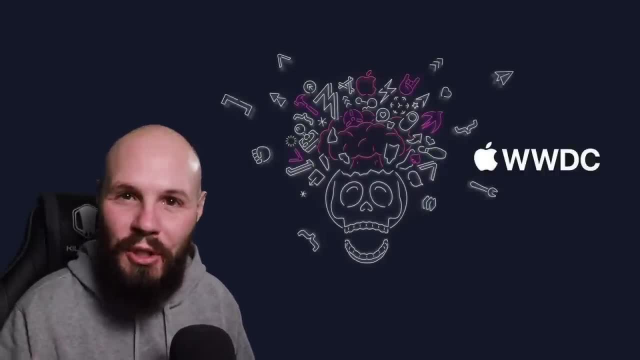 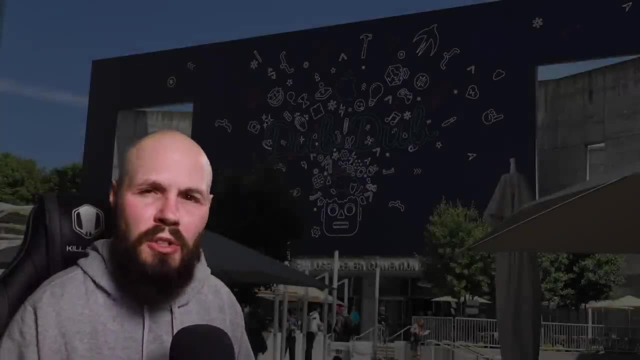 The great thing is, you can experience this in two ways. one, if you're lucky enough to go, which is like $1,600, at least as of 2019, for a ticket, and you know you have to win a lottery to even go. It's it's a super expensive trip. 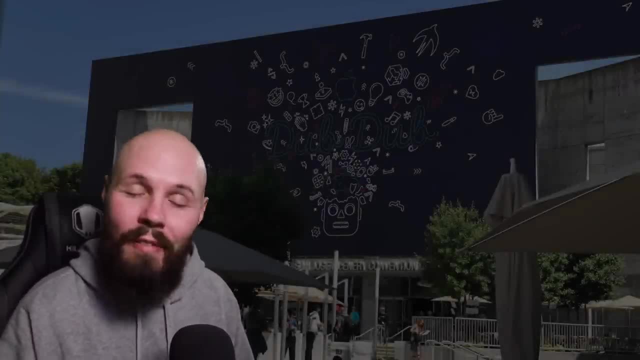 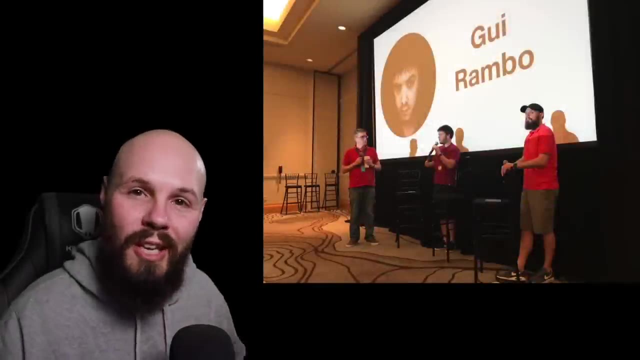 But if you live in the area or you can make it and you know it, you have the money. I would recommend going, as it is a great time right. iOS developers from all over the world Converge on to San Jose, California, And it's also a great place to like meet developers you may have been networking with on Twitter or content creators. 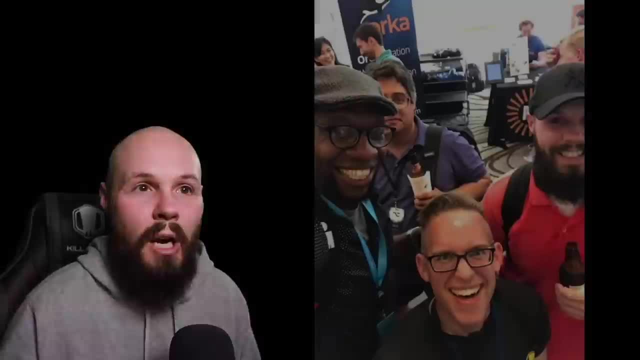 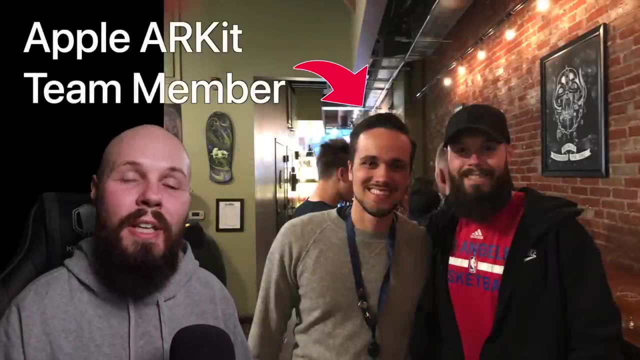 You like, like another weird flex, I know, But like, I took probably a hundred plus selfies- 20 WWDC 2019, like it's. it's just a cool place to go actually meet people that you've interacted on Twitter with all year. Right, because everybody, just, you know, descends on this area. but, of course, 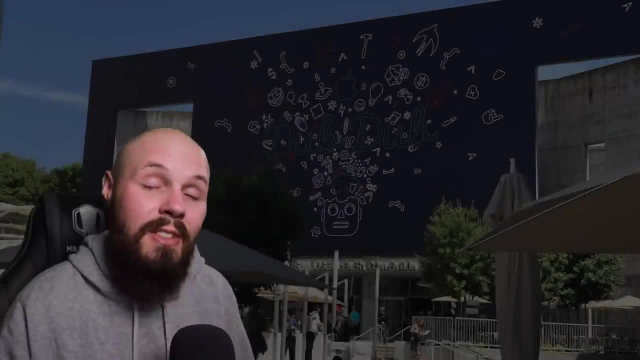 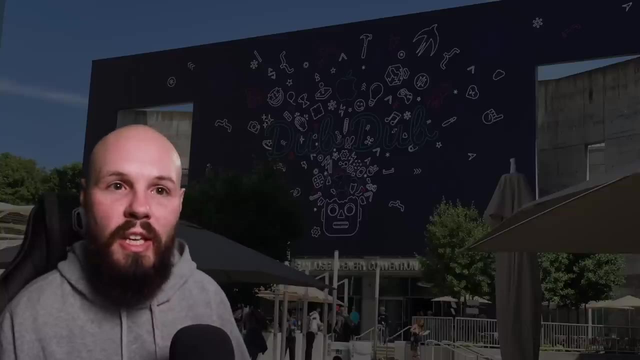 Going to California. getting that $1,600 ticket like that is expensive. totally get it. The bright side is that Apple live streams every single session, and a session is like when they're introducing a new topic, like, for example, when they Introduced Swift. like that was a session and they. 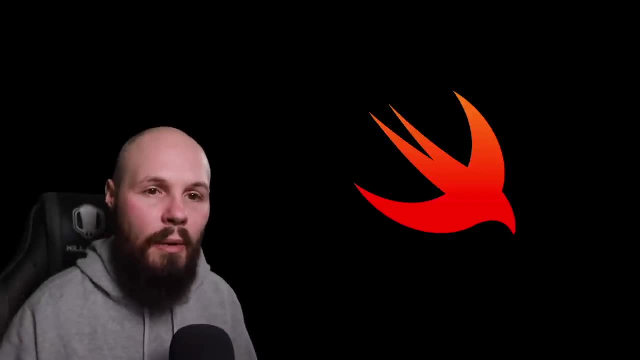 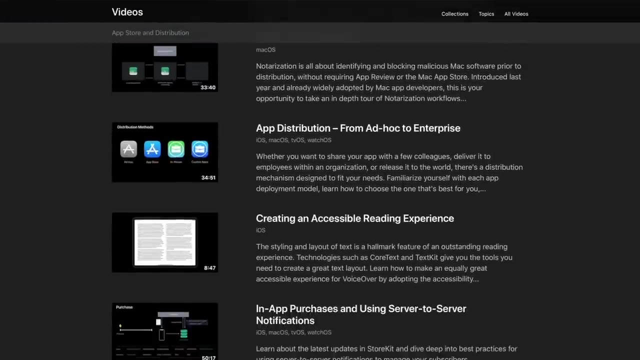 Always do like a what's new and Swift, where they talk about the new stuff coming out. There's over like a hundred sessions, Usually about a half hour to an hour long, and they're all available through the Apple developer app that you can watch on your Apple TV. 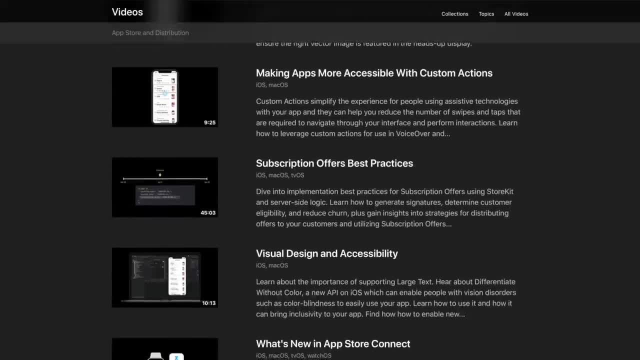 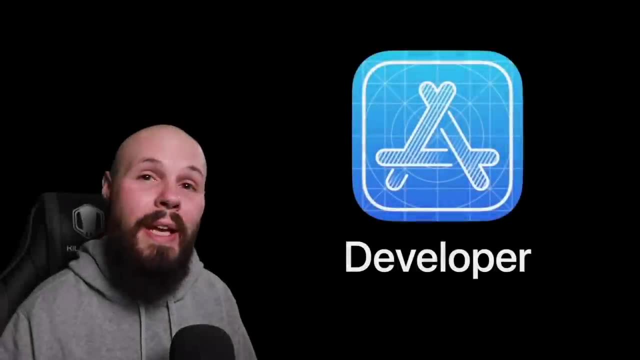 on your phone, on your iPad, so, Literally like the whole month of June, I'm just watching WWDC sessions, like not watching any TV, just catching up on dub dub. So, like I said, even if you can't make it in person, you can still experience it because, also, like, aside from watching all the sessions, like Twitter is. 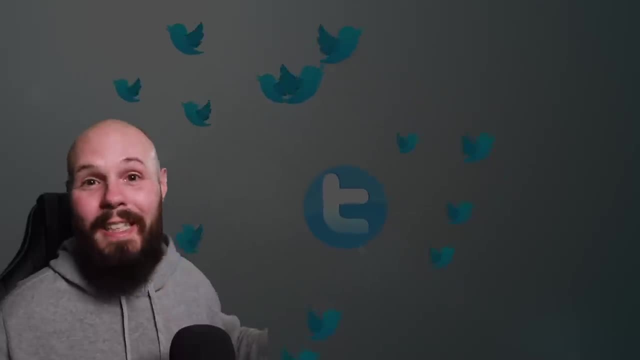 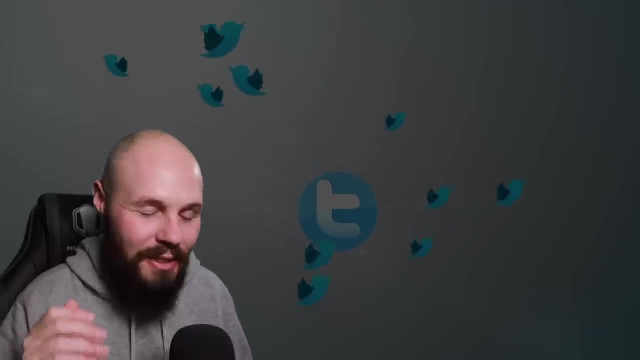 Just a buzz. like iOS dev Twitter Is a party. during that time, everybody's tweeting out stuff. They're playing with the new frameworks, playing with the new toys, tweeting out their opinion on the new features, like it's just. it's just an awesome Time of year as an iOS developer and it's funny, like every year. 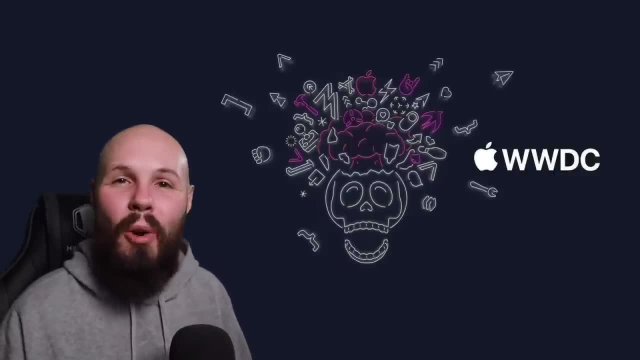 I try to say like I'm gonna watch every session because I get so pumped. I usually end up watching about 30 to 40 of the sessions, But it's literally like like whatever your favorite TV show ever is, it'd be like if they just dropped four seasons on Netflix. 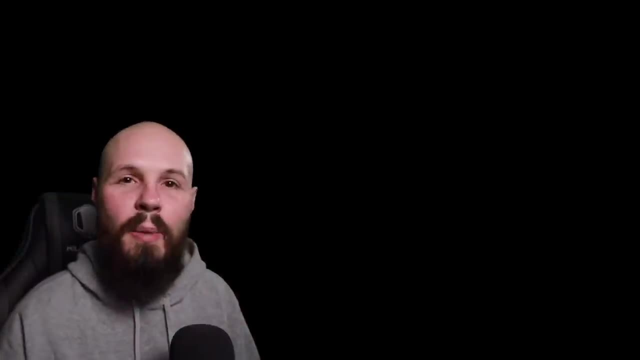 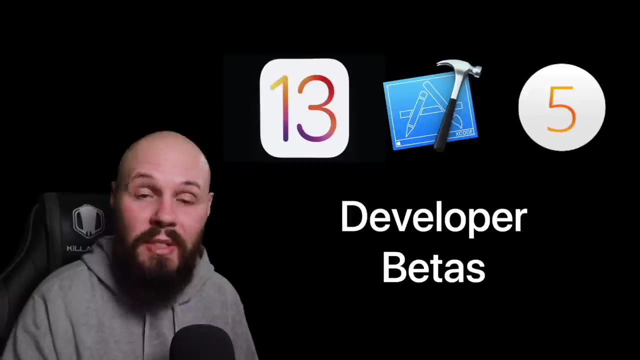 And you just get to binge it right. that's pretty much what it's like. now Let's talk about the betas. I know I touched on it a little bit before, But you know there's betas for iPad OS, iOS, Mac OS, watch OS, basically every platform Apple has. they release the betas and 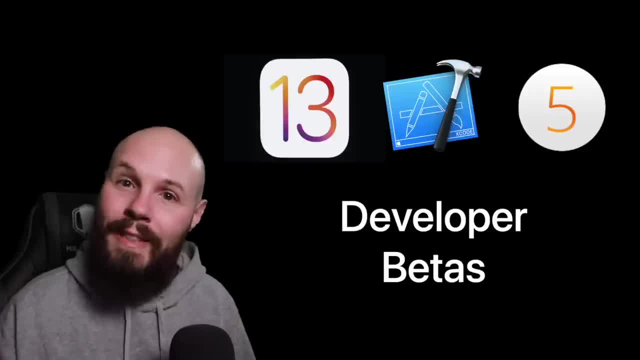 It's not wise to go download the betas on what we call your daily driver. That means the phone you use every day, the one you need because betas are buggy. betas will crash all the time, Especially like a Mac OS beta. maybe some programs you you need won't work on the new beta. so 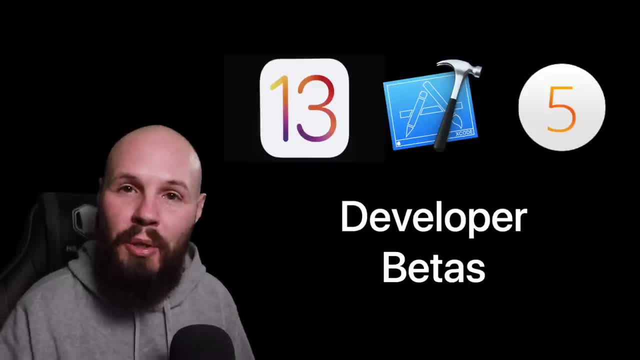 Don't download the beta unless you have, like a spare device that you can put it on to test things out. But the whole purpose of these betas, even though, like I think, most people use it just to play around with the new toys before the general public. 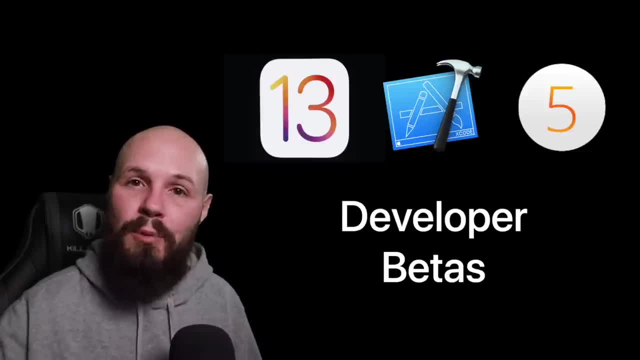 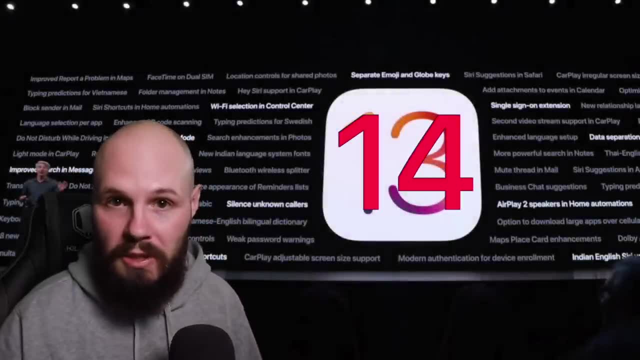 Gets to is that it's to help developers get their apps ready for the new iOS release. for example, this September, September 2020, iOS 14 will be released. We don't know anything about it yet, but you know, if there's big features, Developers have to get their apps ready. So when it's officially launched in September, like their apps are ready to go. 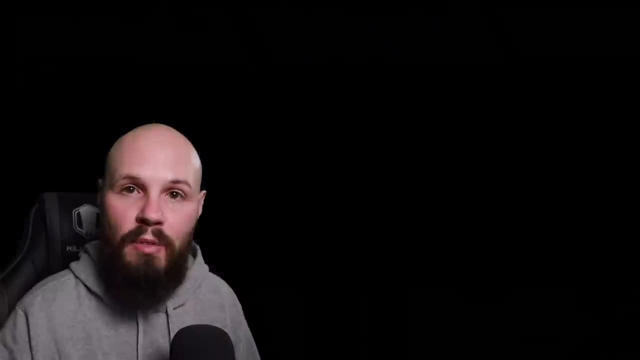 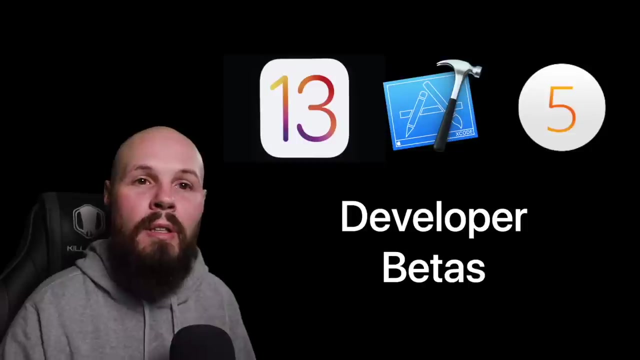 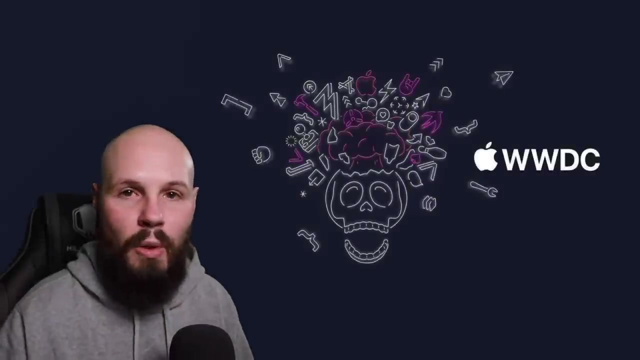 So what happens is developers Update their apps from June to September On the betas. they get all the new features ready that way. again, when the new iPhone event- that happens in late September- and iOS 14 launches, Their app is all updated, ready to go on day one. Now This course is coming out in March of 2020. 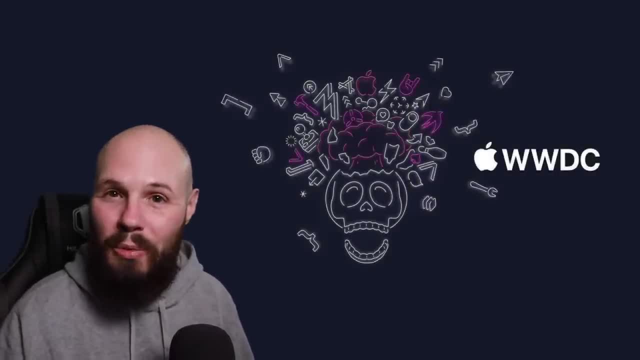 So, if you're watching this, like right away, WWDC 2020 comes in June, So it's right around the corner. So let's talk about, like, how you can learn as a brand new iOS developer. Now, Here's the thing, not gonna lie. 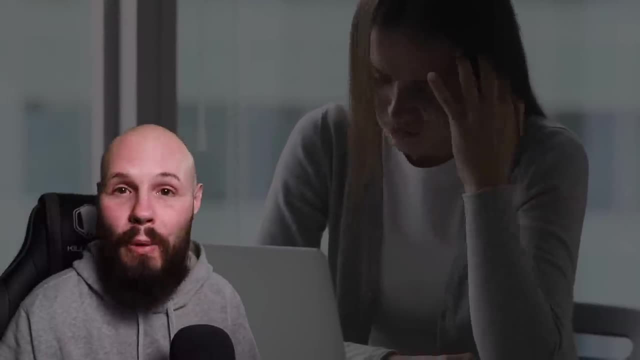 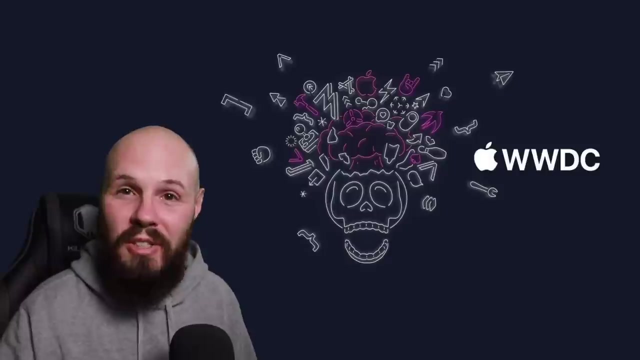 It is going to be Overwhelming for a new iOS developer. Like I remember my first WWDC, which was 2015, I was excited, I got caught up in it. But when watching the sessions and, you know, trying to follow on Twitter, reading the blog post, you know hearing people's opinions. 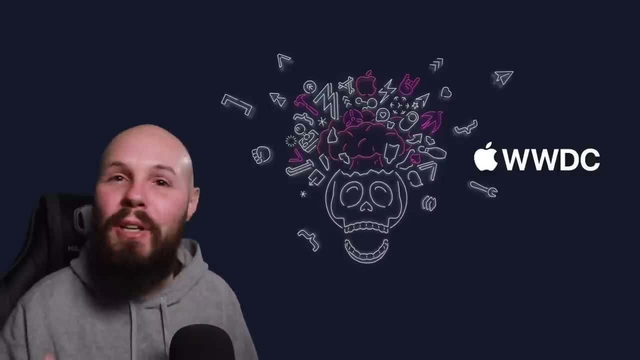 I had no idea what they were talking about, like I maybe understood five to ten percent of it. the other 90% Right over my head. That's fine, Like I. I still am glad that I did that because that exposed me to everything I was able to immerse myself. even if I didn't get it, I was still hearing the terms, I was still 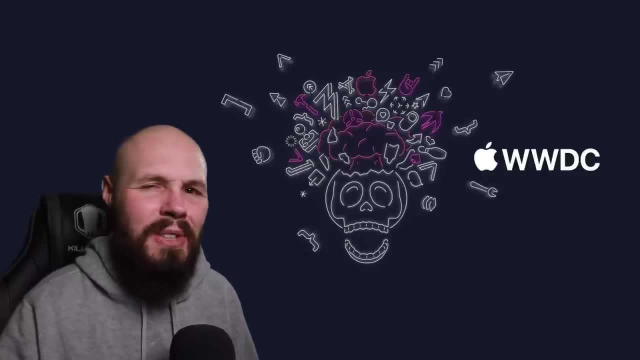 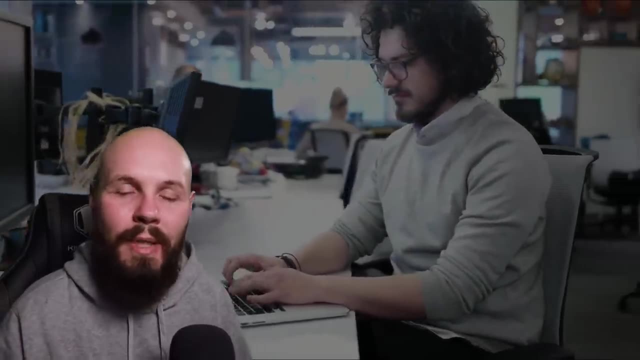 You know learning about. you know things that existed. even if I didn't understand how it worked, I still knew it existed. and over time, as you're hearing this stuff It just it starts to like sink in over time. But again you got to immerse yourself. 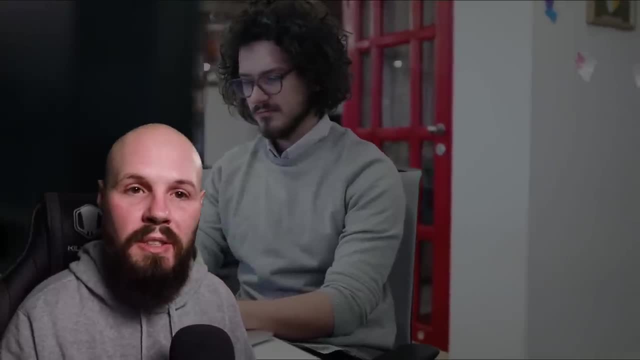 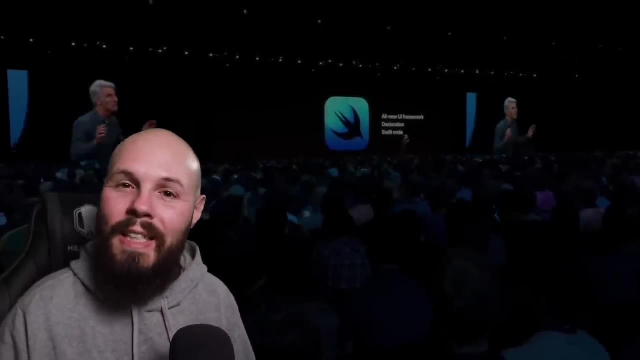 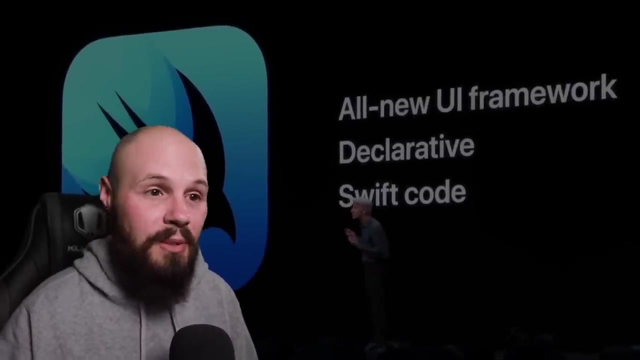 So even if you feel intimidated, your very first year of WWDC it's, I would still watch it, still go through it again. I didn't understand almost any of it, But the good thing is that gets better. like my next WWDC, I understood maybe 30 to 40 percent of it and then by the third year I was like all in. 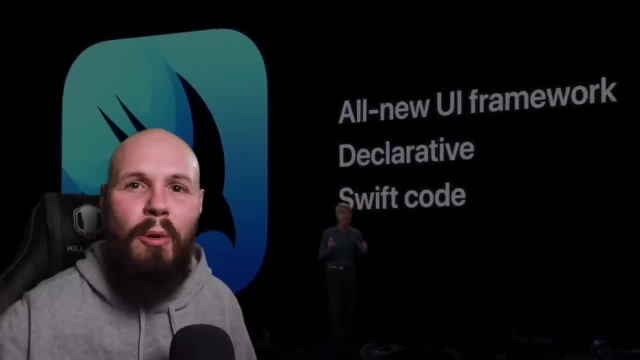 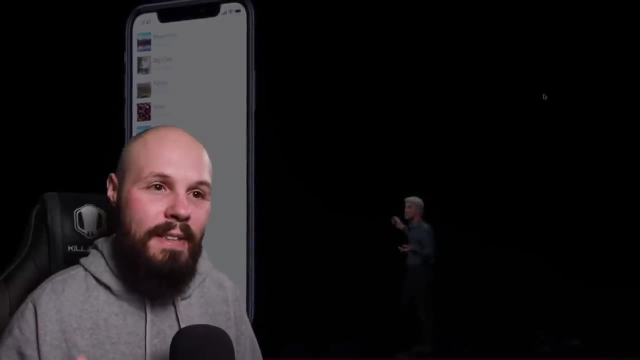 Obviously, you don't understand everything, because they're talking about. you know frameworks and api's that you never use, But, like I understood the lingo, when they put code up on the screen, I knew exactly what was going on. It's it just it gets better and easier, and then again by your second or third year, like dub-dub is gonna be your favorite time. 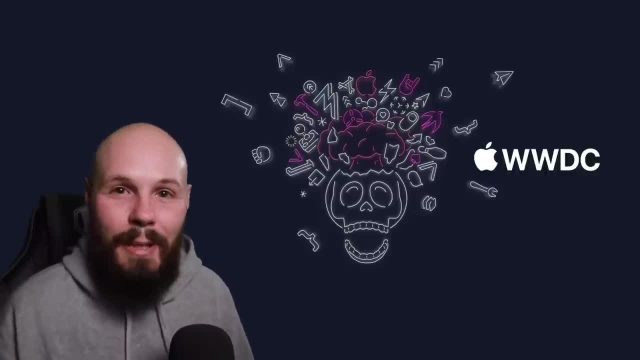 Of year. it's going to be awesome. It's just you can tell I'm excited just talking about it. So in this video I just wanted to let you know what WWDC was, why it's so exciting, how you can learn from it And, like I said, the keynote is kind of like the highlight of the event. 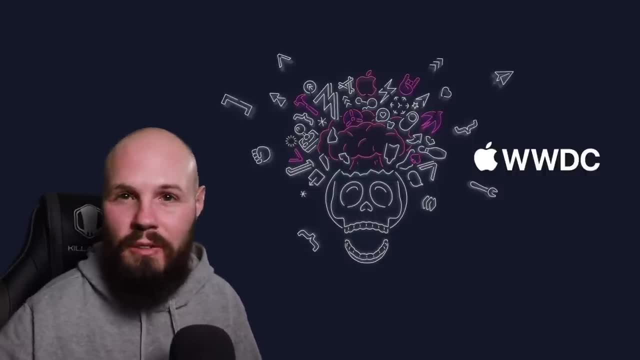 That's what kicks everything off. It's like a two hour long keynote and they're showing off all the big picture Features. like to be honest with you, like the keynote can be watched by like non developers, because it's really like: here's the new features in iOS 14. 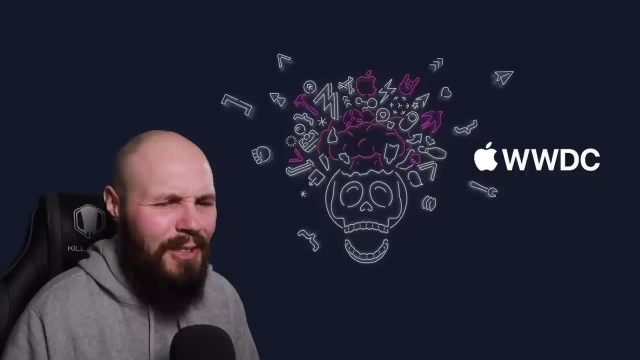 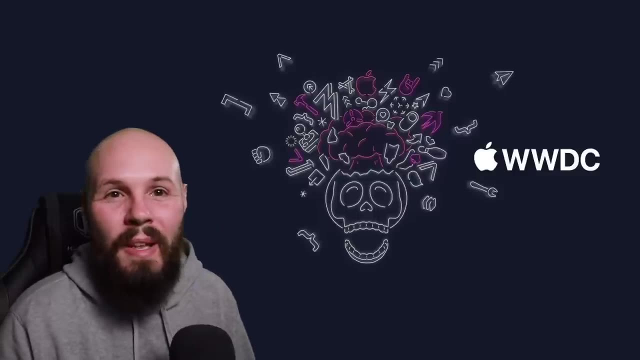 However, every other video is basically for developers. But yeah, just just like try following along Twitter during the keynote. It's just, it's going too fast to even keep up with, but it's so much fun. So if WWDC 2020 is going to be your first one, you know we're gonna be in slack, you know. 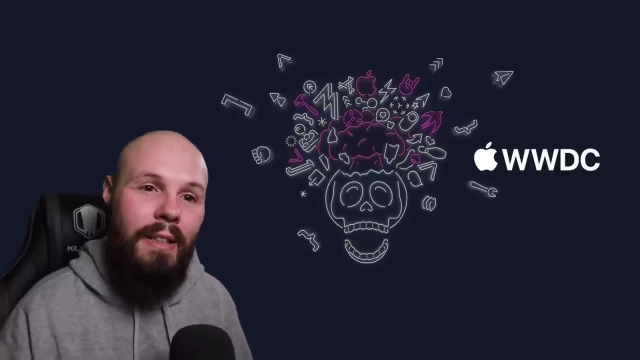 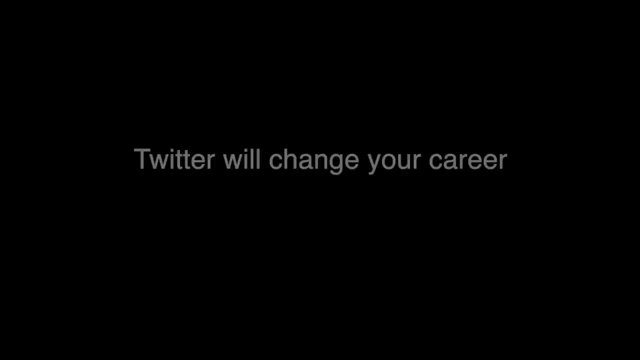 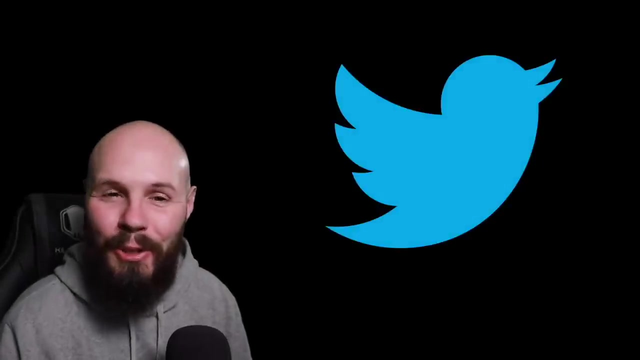 We have a slack group for this course. I'm sure everybody in slacks going to be talking about it. It's just a fun community event. again, It's the best time of year, So I hope you enjoy your first WWDC- If Twitter isn't the most valuable thing in my developer career. 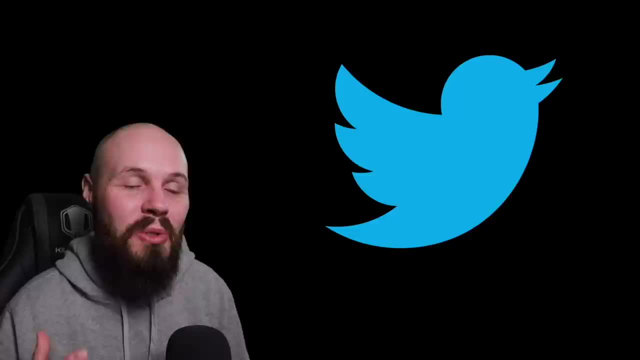 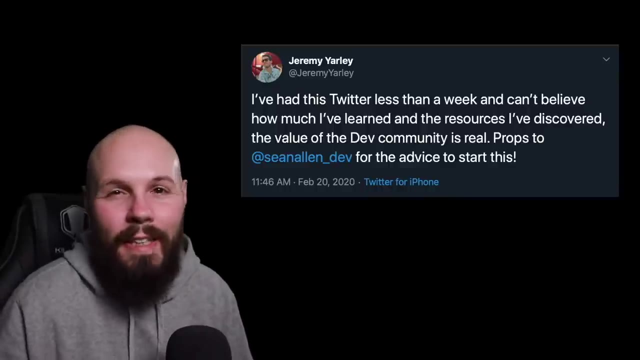 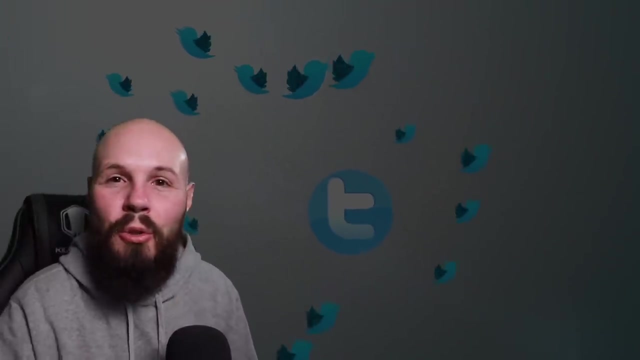 It's definitely in the top three and that surprises so many new developers. And I know Twitter gets a bad rap. all the politics, bullying, cancel, culture, Like I get it, Twitter can be bad. but the thing about Twitter is You kind of control what you see right, like based on who you follow, like that's what you're gonna see. 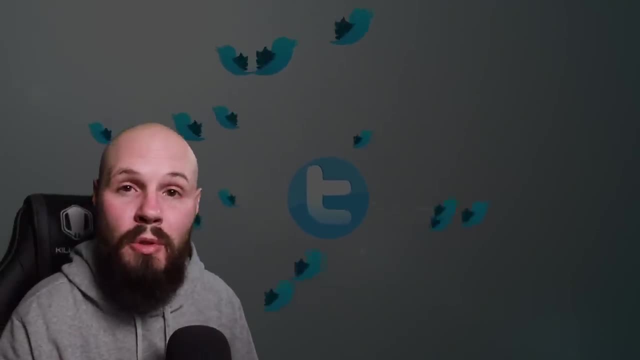 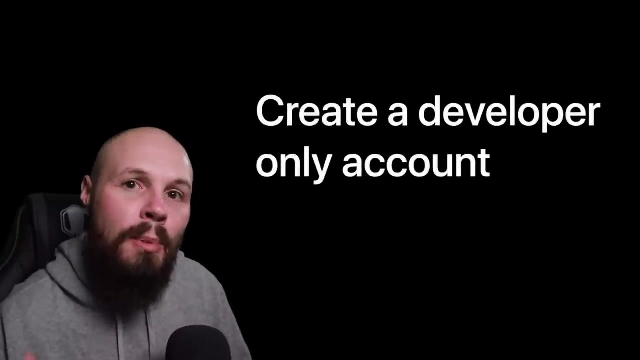 So if you focus a Twitter account- and I've even seen people do this right- They have their personal Twitter account for all their hobbies or whatever They're into, and then they create a special developer account and that's like their professional account, where all they do is follow developers. 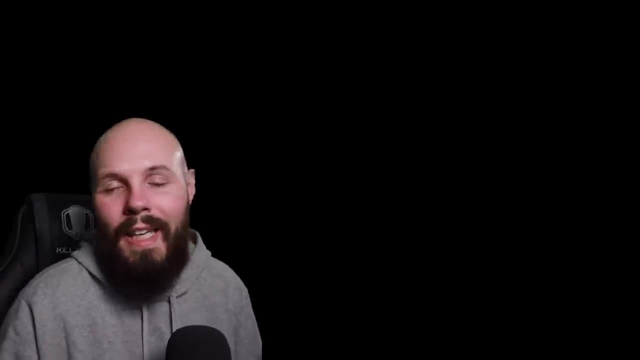 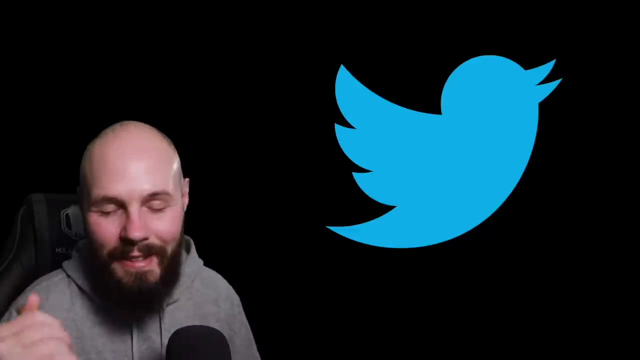 That's how they interact with the developer community, etc. So, like I said, I kind of get why you may have reservations about joining Twitter, But I'm here to tell you in this video It's insanely, insanely valuable for developers, and that's because developers pretty much live on Twitter. 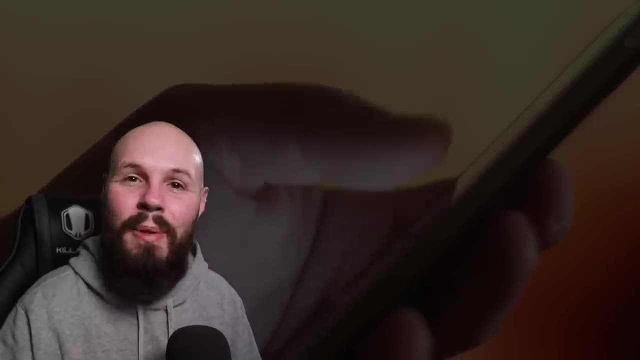 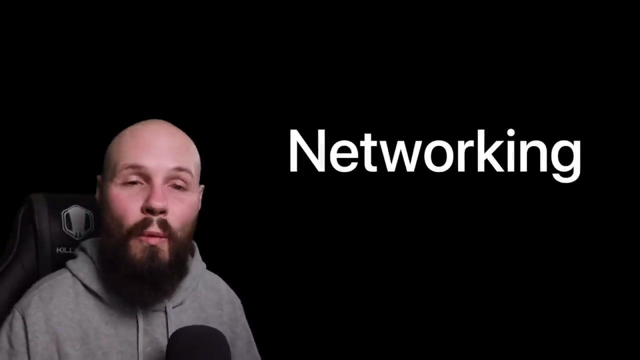 Like, like, almost too much. but the point is is like that's where everybody hangs out in the developer community. Now, the first benefit of Twitter I want to talk about is networking. It is probably the number one way to network in a developer community, right, Of course you can go to conferences, go to local meetups. 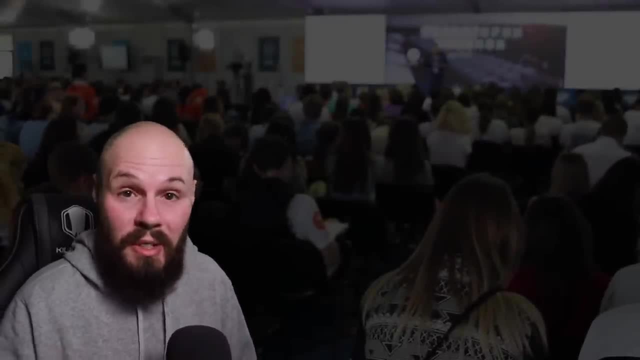 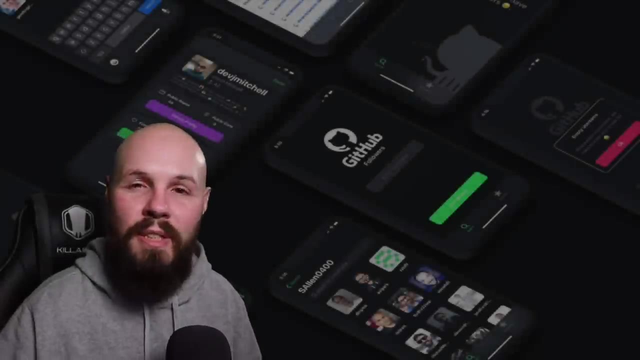 But that's a. that's a small number of people, whereas Twitter is like the whole industry. Let me share a quick story about something that can only happen on Twitter. right, I have another course out, called the iOS take-home project course, where we implement a collection view and we use this new thing in iOS. 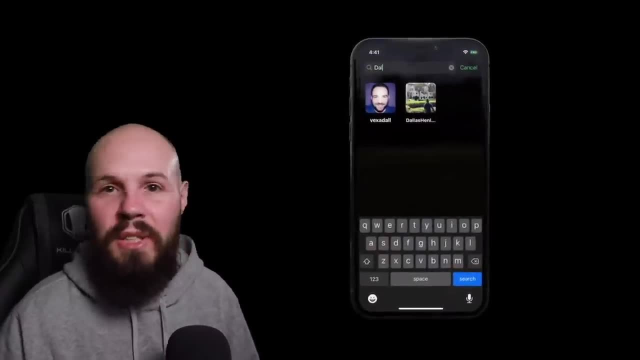 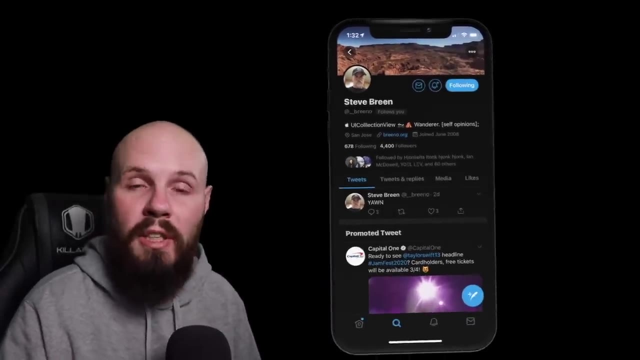 13 called difficult data source. Well, I'm talking about it on Twitter. I'm sharing my work, I'm retweeting other students, you know, tweeting stuff out, and an engineer named Steve Breen, you know, Like the tweet retweeted, the tweet started following me and if you look into who Steve Breen is, 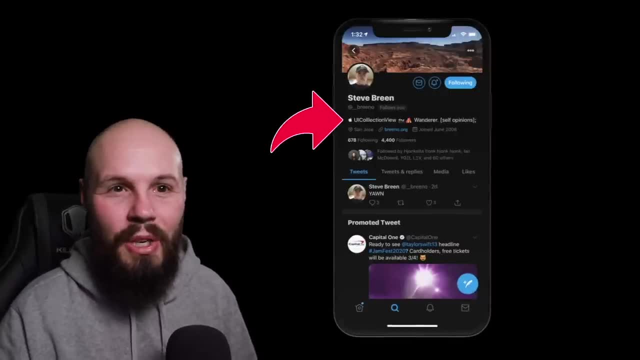 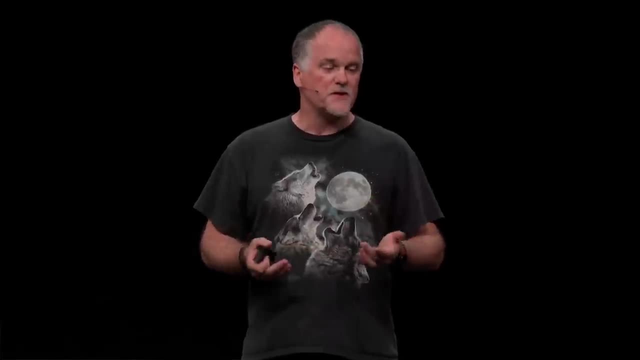 He's an Apple engineer working on the UI collection view team who actually helped build the difficult data source stuff And actually if you watch the WWDC video on difficult data source, He's the one up there presenting introducing this to the world. So now Steve knows about my work. 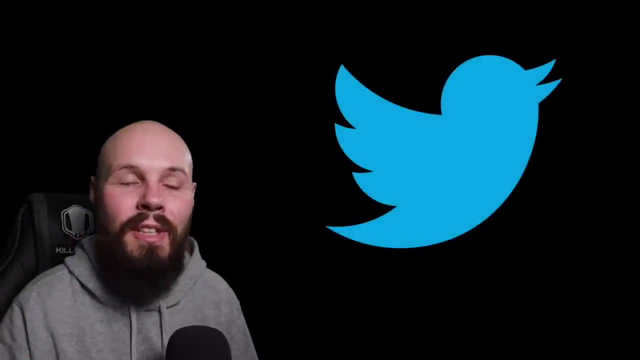 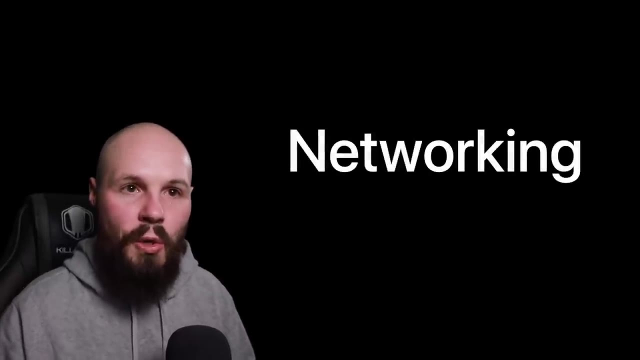 We follow each other on Twitter, We can now interact, and that kind of stuff can only happen on Twitter. So back to networking. right again, Twitter is like the number one way to network as a developer. now, when you're networking, keep in mind that networking is a 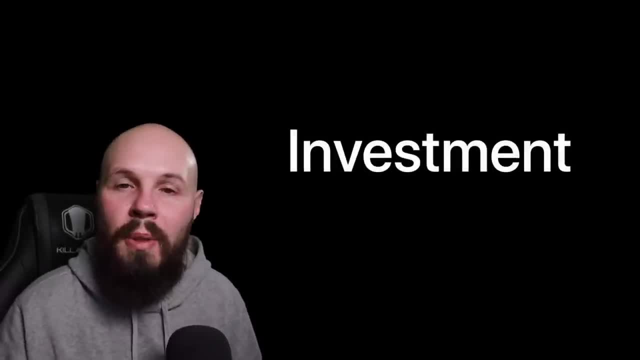 Long-term investment- right. This is going to be something that pays off and you build over years, but that's okay. You plan on being an iOS developer for years, right? And because you're building that over your entire career, Yes, You may want to try to network with. 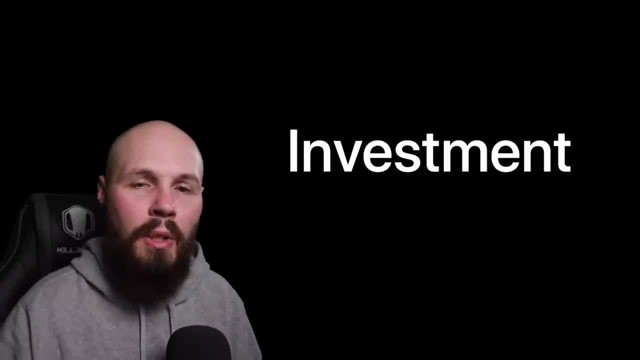 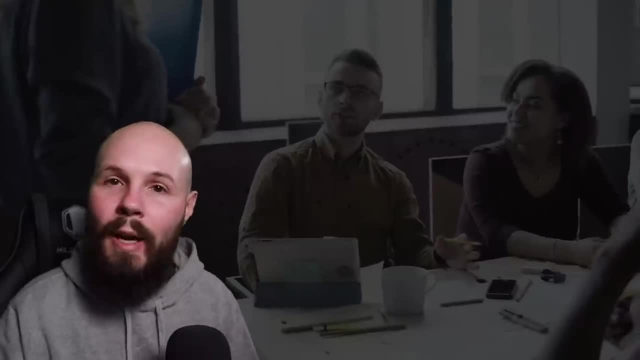 Those Apple engineers over those more senior engineers. but don't forget to network with your peers right now, other developers Just learning like you again. another story: I did my iOS developer bootcamp in 2015- So that's five years ago now- in my peers. 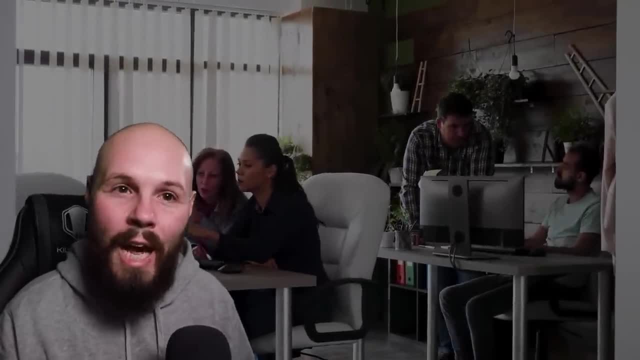 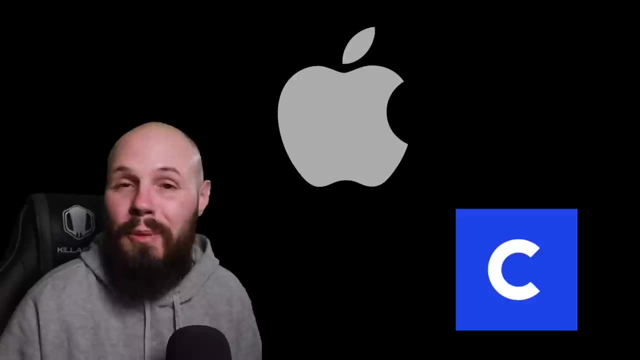 There were just a bunch of students who didn't even really know how to program. Now, two of those graduates are engineers at Apple. another went on to work at coinbase and built the native coinbase app during the 2017, you know, crypto boom. It's just my point is: is your peers right now? 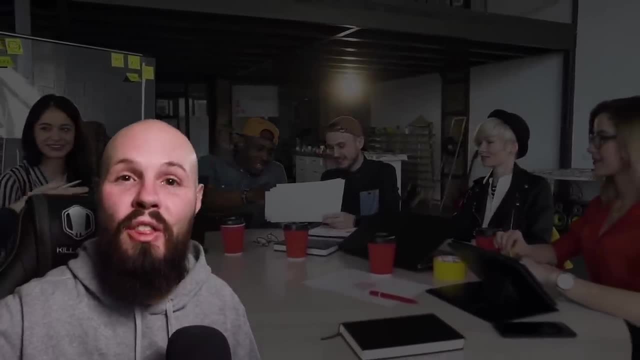 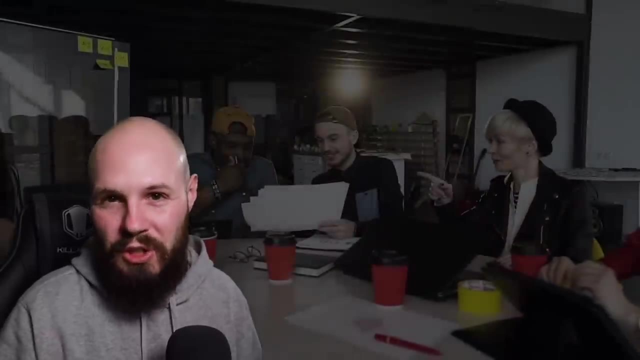 In three to five years are gonna go on to do great things. So if you're building those relationships now and let those build over five years, you know when it comes time to get Probably not that first job right, Cuz they may not be able to help you right away. 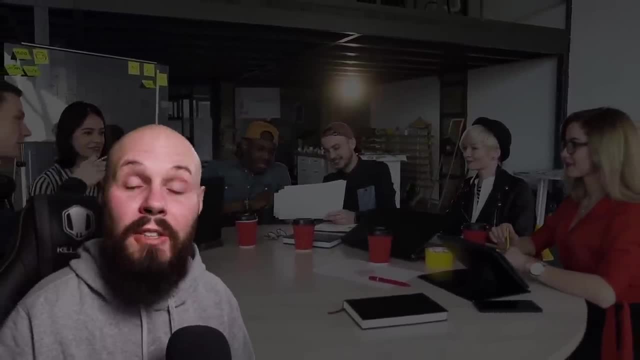 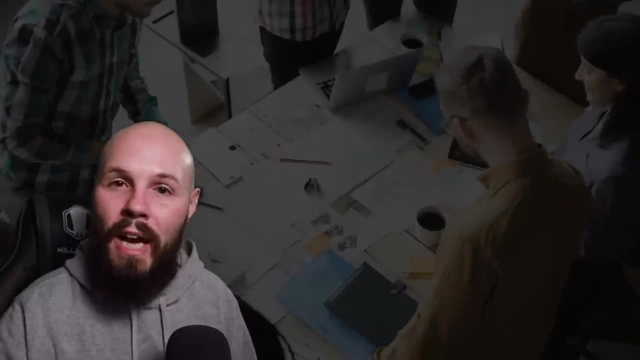 But you know three, four, five years in your career when you're ready to go work at a big company. you know Facebook, Instagram, Apple, Google, YouTube, whatever. now It's very likely that you're going to have contacts in relationships with people on those teams. Now You may be wondering: like well? 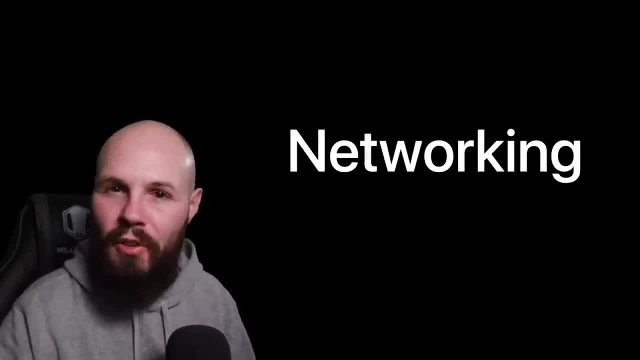 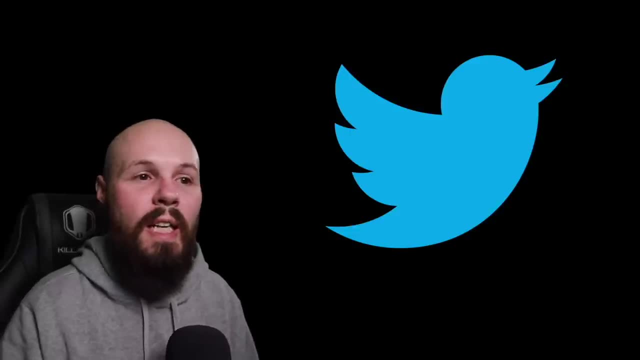 How do I network on Twitter? We're going to get into like finding people to follow later in the video, but at the end of the day, Twitter is just a conversation, right? So if you follow people and you see them talking about something like, join the conversation. 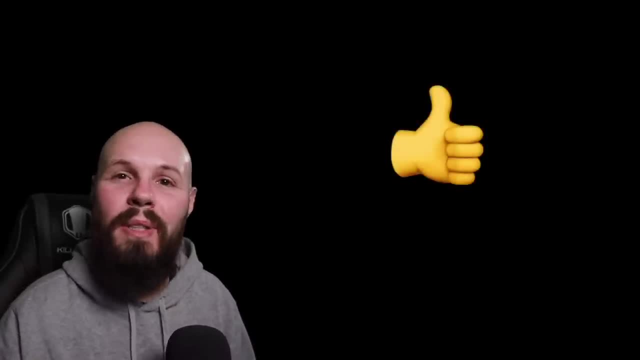 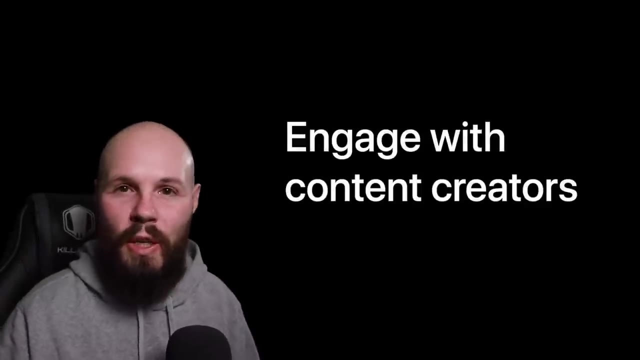 you know, don't just pop in with a thumbs up emoji, but like, actually have something intelligent to say. Or another way is to interact with content creators. content And that kind of leads me to another reason why Twitter is so valuable. If you follow all the YouTubers, the bloggers, the podcasters, right? 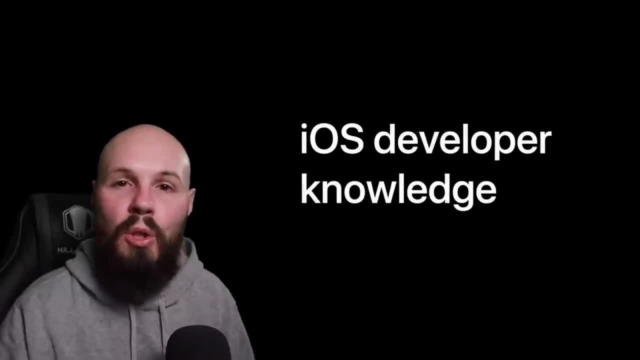 They're constantly putting out awesome swift iOS developer learning material. And how do they share that material? They put it out on Twitter. So if you're following all those people, your feed is going to be a constant influx of new blog posts to read, new podcasts to listen to, new YouTube videos to watch. 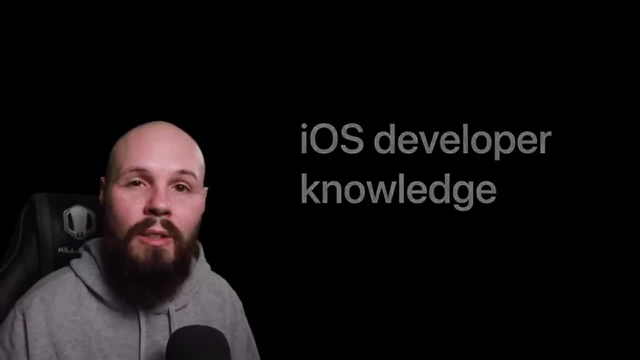 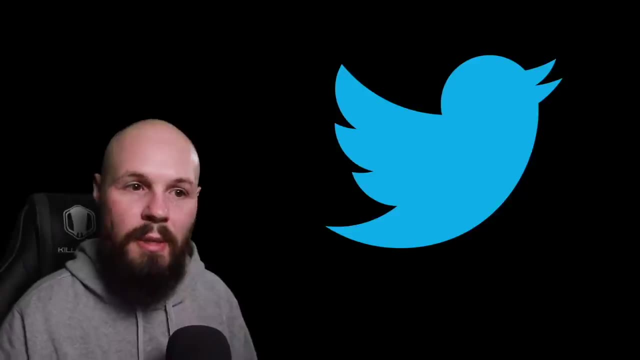 You're going to constantly get knowledge presented right in front of you, So it's a great way to learn as well. And that content presents two opportunities for you to network. One is with the content creator itself. Content creators in this space typically have, like the big ones you know, 20 to 30,000. 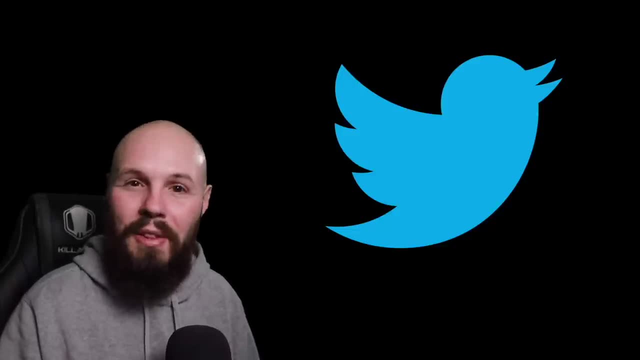 people. Twitter followers may sound like a lot, but as somebody with almost 20,000 myself- weird flex- I know, uh, you're, you're, you're going to get noticed, right, If you retweet my stuff and retweet with a comment or you're always liking, you're always. 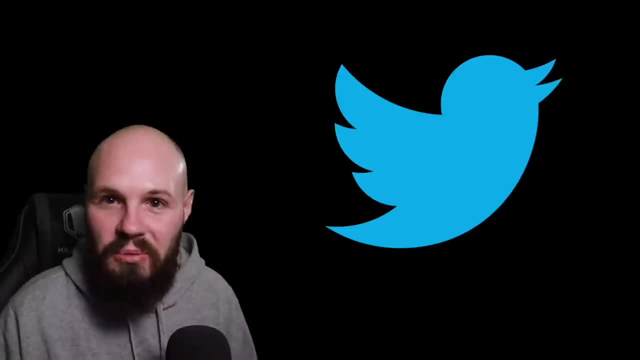 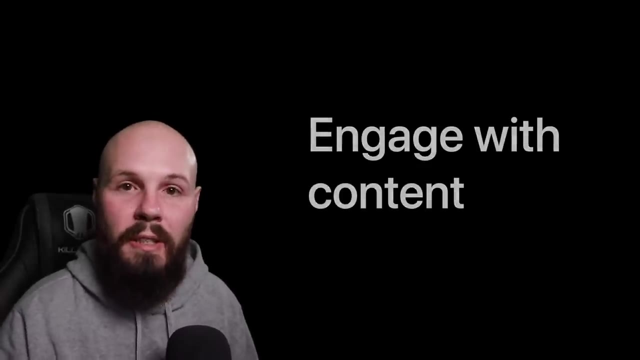 commenting on my tweets, Like I'm not big enough to not notice you, right? So nobody in the iOS space is too big to not notice you, So interact with the content, like actually read someone's blog post after they tweet it and say, Hey, thanks for the blog post. 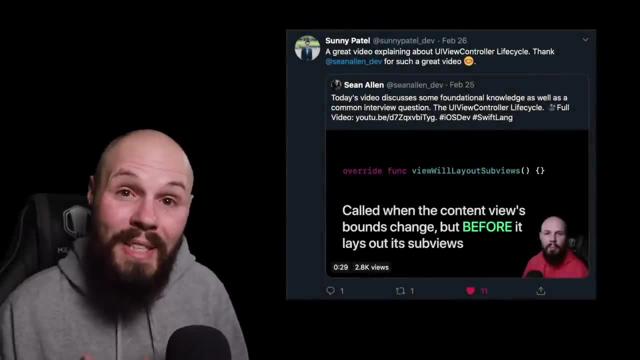 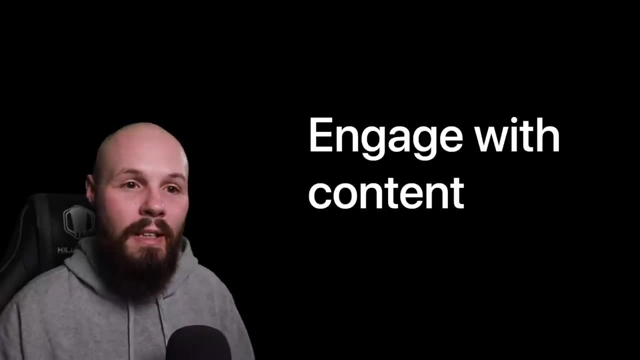 I really liked what you said about this. It really helped a lot. Thanks, Like. that means a ton for the content creators And if you're constantly supporting them, constantly retweeting their stuff, constantly commenting, they're going to know who you are. 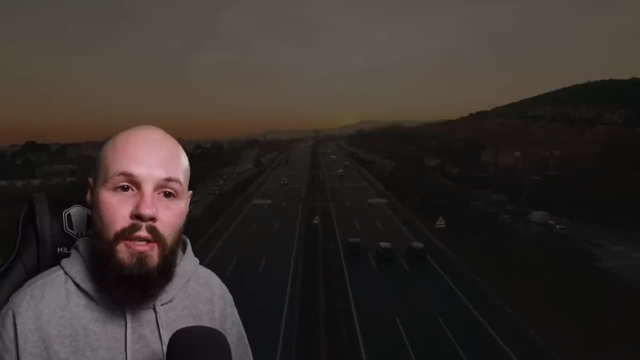 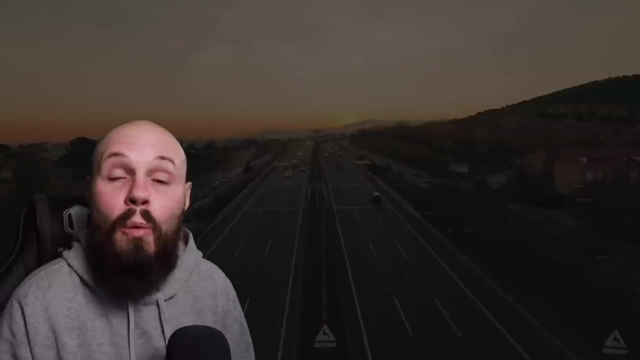 And again, that's just networking. It's a two way street, right. The content creator gave you valuable content, helped you learn. You help them out by sharing their stuff and interacting and engaging with their content. Like that's how networking works. 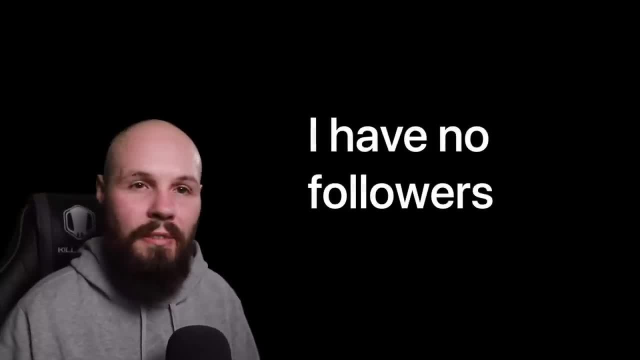 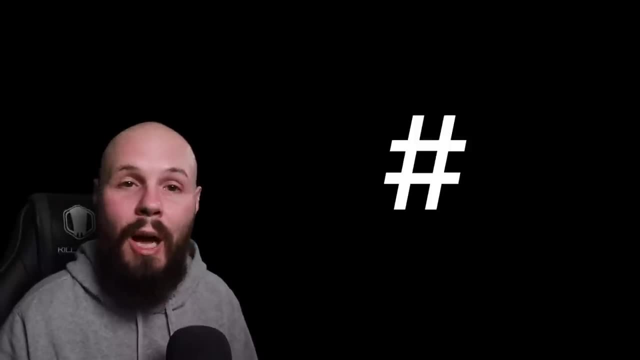 It's a two way street. Now you may be thinking: well, what good does a retweet do if I have seven followers? right, I get that. That's the power of hashtags. come in, So still retweet it. you know, maybe retweet it with a comment on it and then make sure. 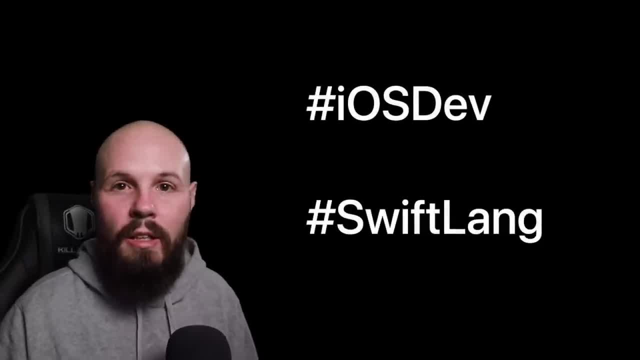 you use hashtag iOS dev or hashtag Swift slang. Those are the hashtags that people search in this community. So even if you have no followers, when you put the hashtags on there, that content can still get discovered and you're helping the content creator share. 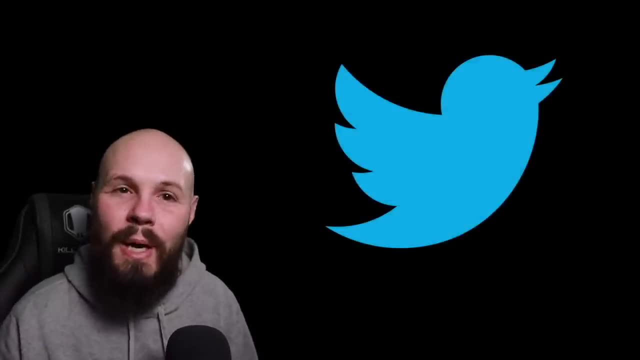 And again, this is not about Hey, you should help content creators. Again, this is about networking to the point where you can build a relationship with that content creator, Cause I can tell you firsthand, I know developers and have built relationships with developers. 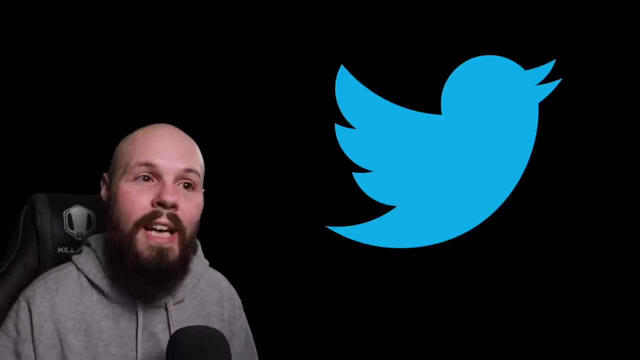 because they've been sharing my stuff for years now. And I'll tell you what. if they ever asked me for a favor or needed help for something or needed a recommendation for a job, I would go way above and beyond for them, because they 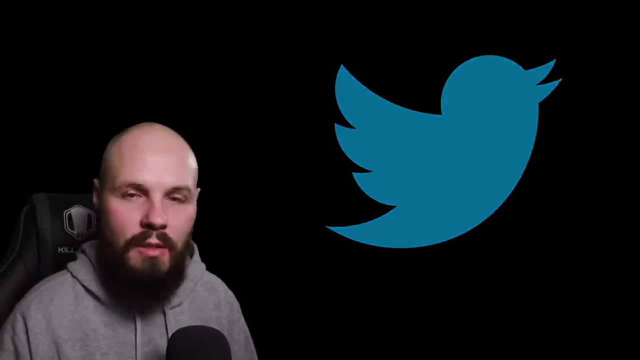 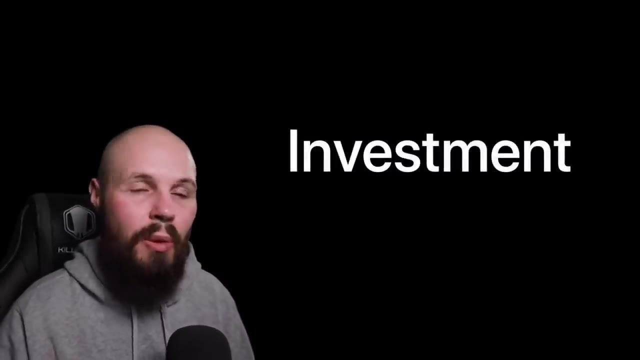 have been supporting my work for years. Again, it's a two way street. So back to the benefits of networking. Remember, I want to stress this: This is a long-term investment, right? You can't just reply to a couple of tweets and then, in a month later, be like: ah, networking. 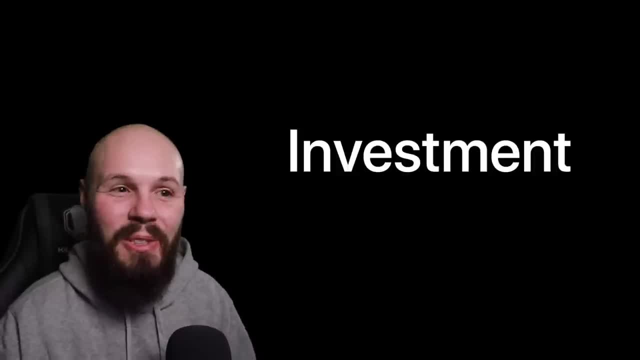 doesn't work right. I didn't get a job from it. That's not how it goes. This is going to pay off one, two, three, four years down the road. Again, if you've done networking correctly, over after three, four years you're going. 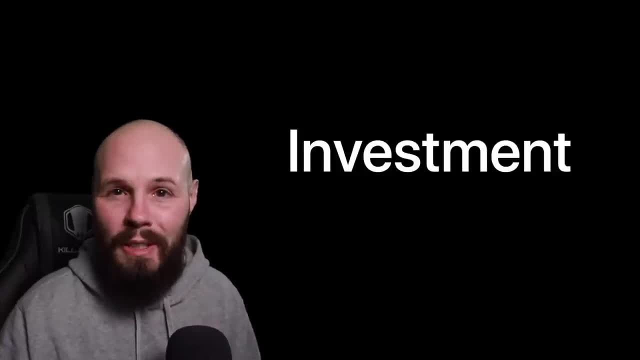 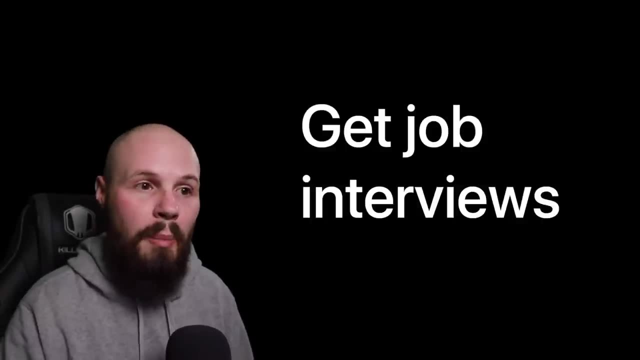 to have contacts at Basically every major tech company out there. That's how I used it right. I built up my network and my contacts mostly through my YouTube channel, But when it came time for me to like start interviewing at big companies, I didn't go. 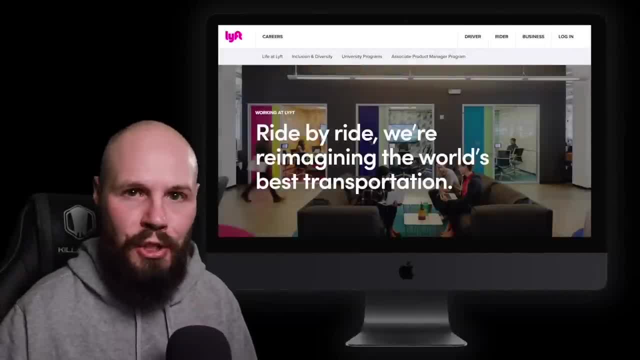 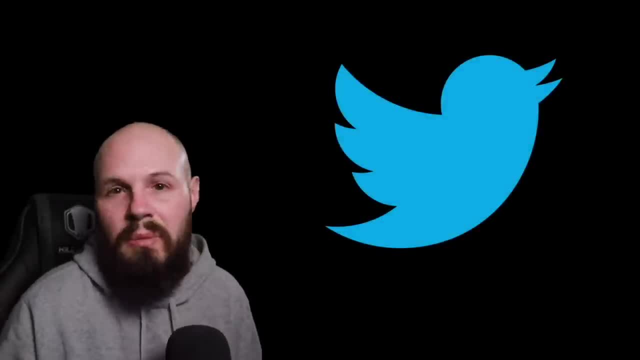 to the website and apply. right. I didn't go to lyftcom slash jobs and fill out an application. I went to Twitter, went to my contacts, said Hey, so-and-so I'm interested in interviewing at Lyft. I'm just using Lyft as an example. 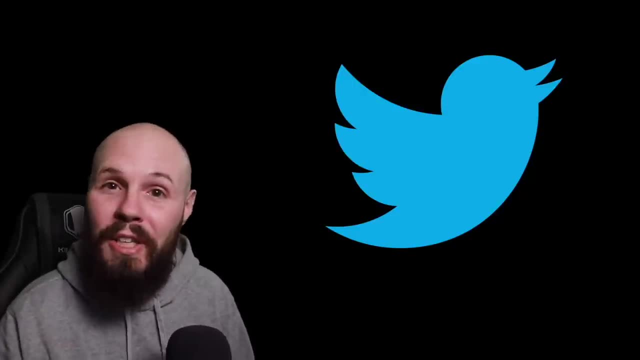 You know, would you mind passing on my resume? After you've built that relationship over a couple of years, they're going to be more than happy to do it, And you're doing it that way Pretty much get you a guaranteed interview. 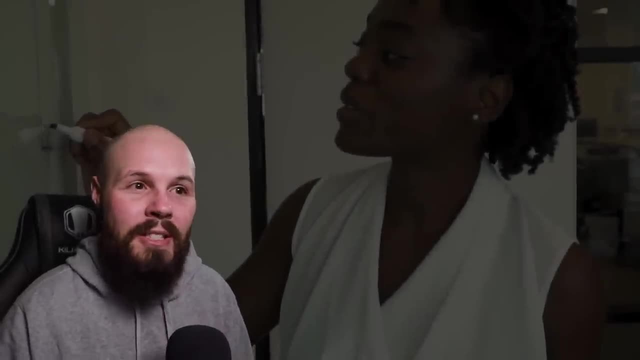 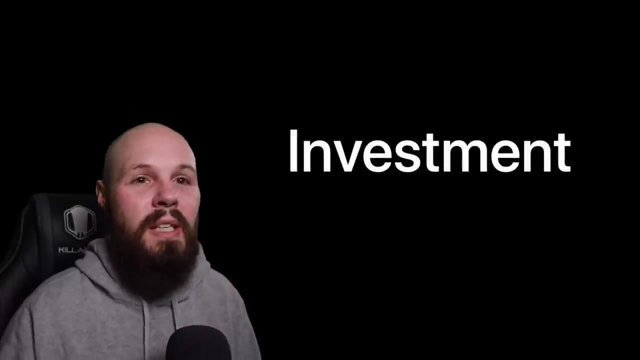 Now, of course, once you're in the interview, it's up to you to perform. but that's how, once you build a network, you can pretty much get an interview at any company like, as long as they have an opening. So that's where the value comes in. 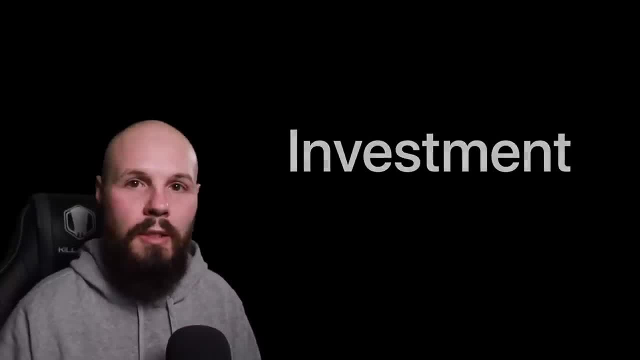 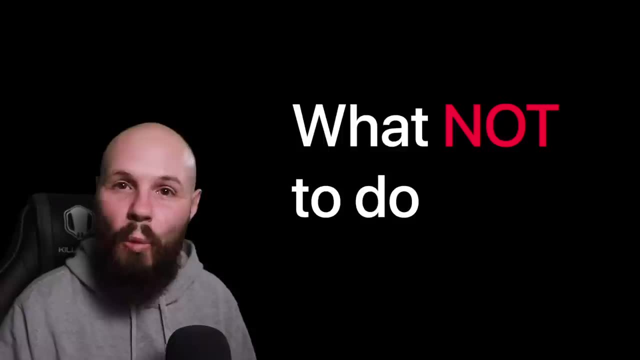 And again, that doesn't pay off till one, two, three, four years down the road. So let's talk about some ways like not to network, right? So definitely get in there and ask questions. you know, feel free to tag one person and 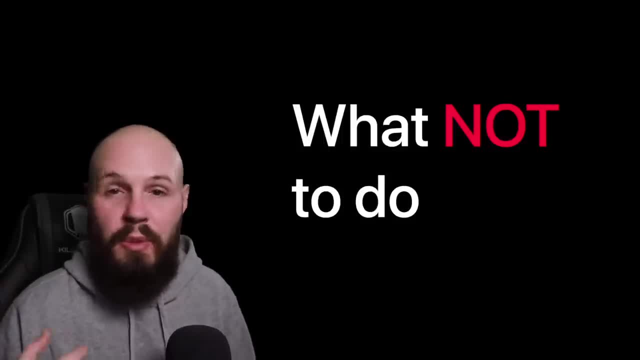 ask questions, but you need to be courteous of that person's time And I'm speaking firsthand, Right? Okay, I get this all the time. A lot of times people will tag me and then they'll just copy and paste a huge view controller. 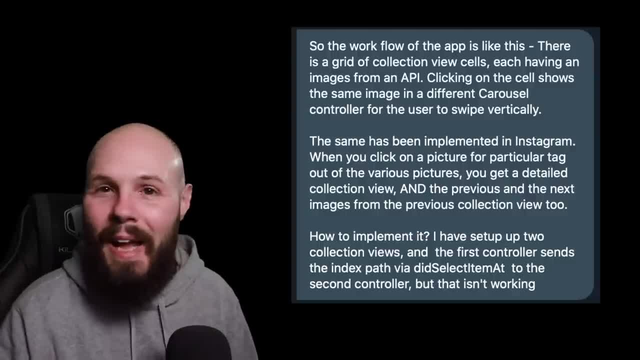 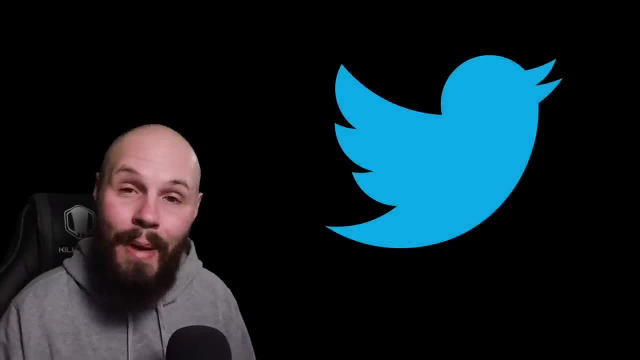 Hey Sean, can you fix my bug Like that's? that's not how you do it, But if you ask me a question on Twitter and you tag me and it's something I can answer off the top of my head and like five minutes, I'm happy to give you a valuable, insightful 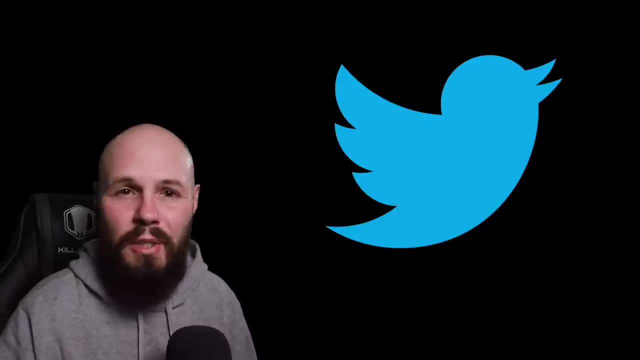 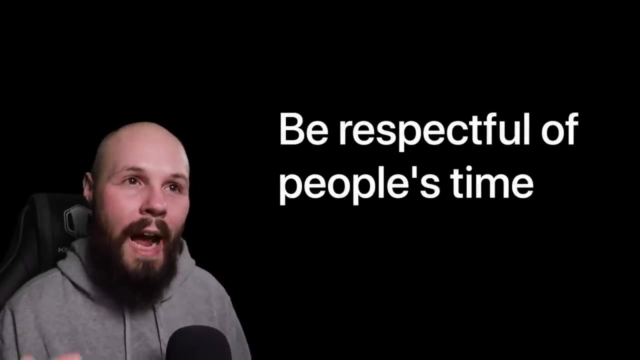 response. you know career related to questions. uh, maybe how to solve a simple problem if you're stuck like that's how you do it again. So when you're asking a question on Twitter, be respectful of their time and think okay. 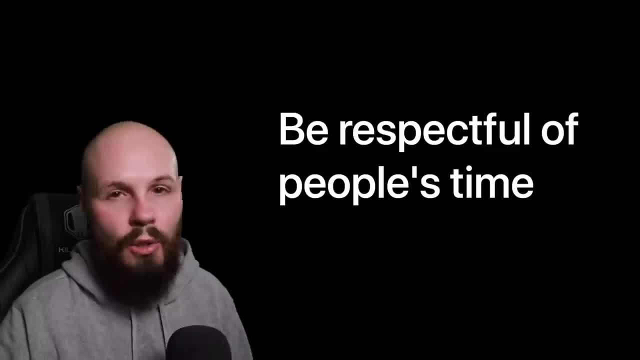 how long is it going to take them to answer this? And if it's short, you know, go for it. If you've got a copy and paste code and they got to read it and try to fix your bug like that's not how you do it. 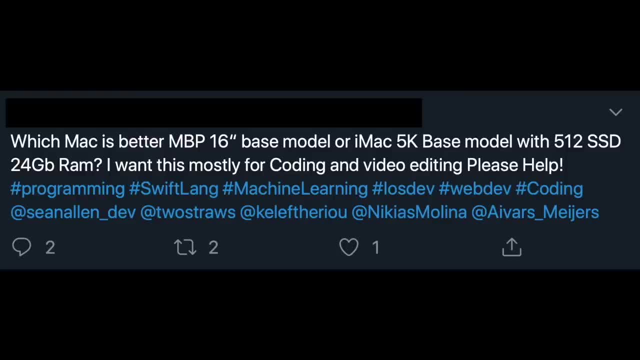 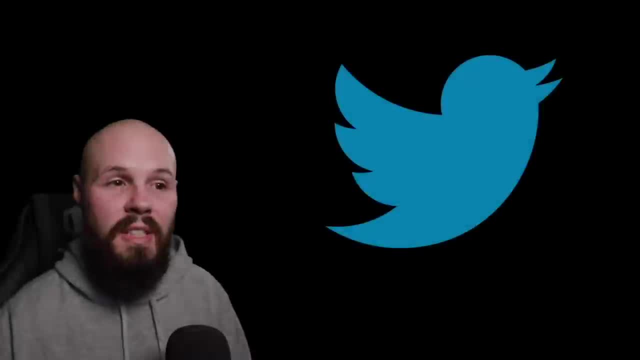 Another thing you don't do is don't ask your question and tag 10 people, right, I see that all the time Somebody will have a question and they'll tag all the top content creators in the iOS space. All that does is that just spams that person's mentions, as people are replying to that. 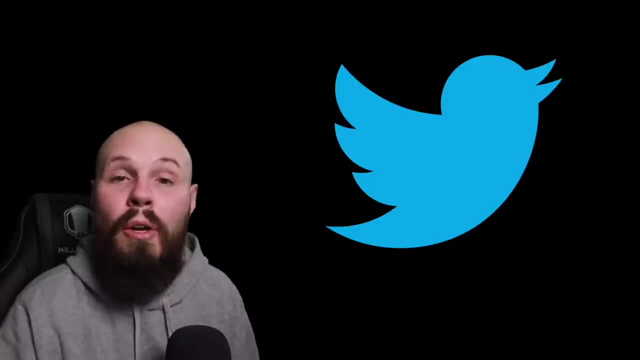 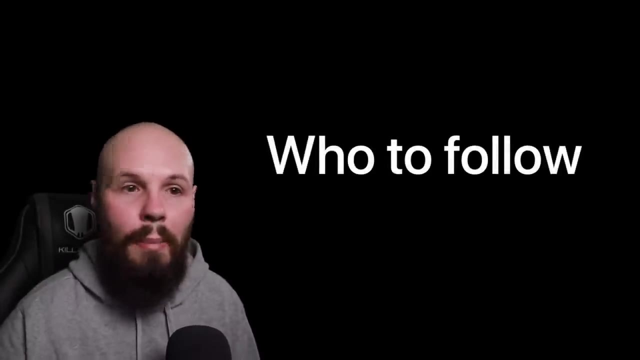 Right, So that's just not a good look. That's more, you're annoying. You're annoying who you're trying to get help from, And that's never a good thing. Now let's talk about like who to follow. First of all, down in the description of this video, I'm going to list a handful of. 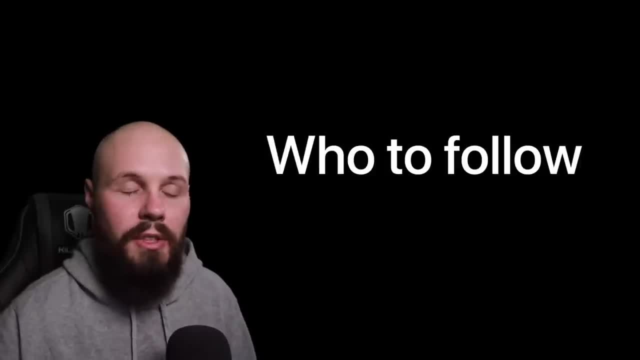 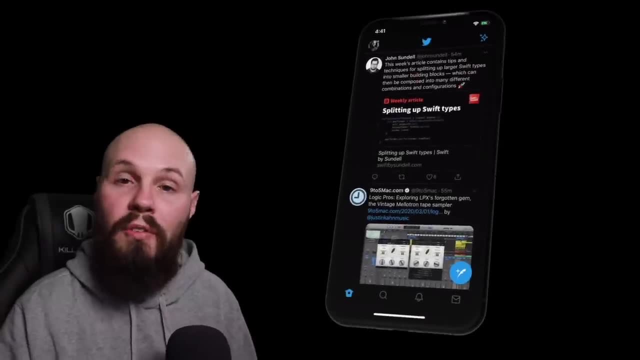 a must- follow Twitter accounts in the iOS dev space, but you're going to need to follow more than that, And there's two main ways to do that. One is to see who those people are following. For example, if you go to my account, you can see who I'm following. 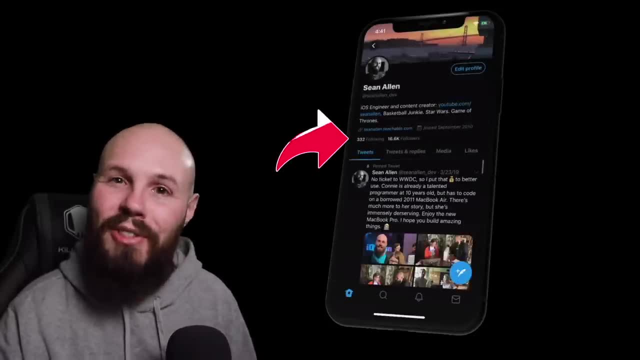 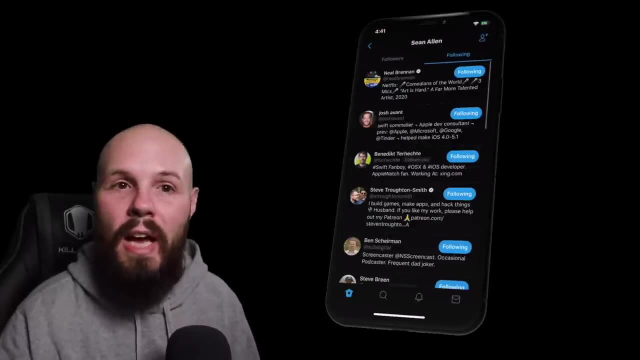 Go down that list and follow the developers you find interesting. Now you're going to have to sift through some like sports stuff, some comedy stuff, some crypto stuff- but it is mostly developers- and then follow the ones you like and then repeat that with other developers. 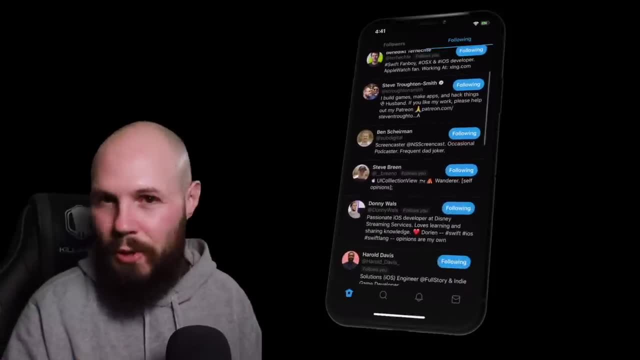 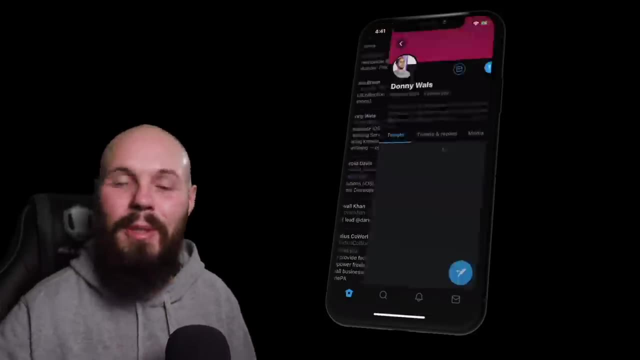 See who they're following, So you can quickly build up Your list. Now here's the trick, though: When you quickly build up your list like this. not all developers like to tweet about developer stuff, right? Sometimes you may follow a developer and you may find 90% of the stuff they tweet is stuff. 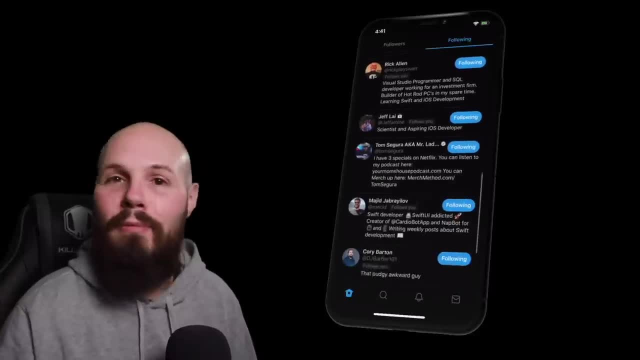 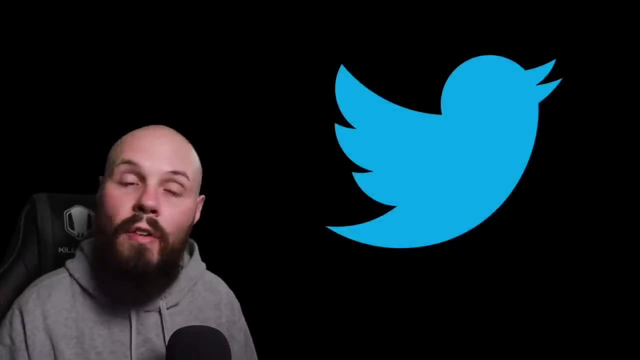 you don't care about, And 10% is developer stuff. Well, you don't have to keep following them. So I guess what I'm trying to say is this is probably going to be a process: You'll end up following a bunch of developers and then you may end up having to unfollow. 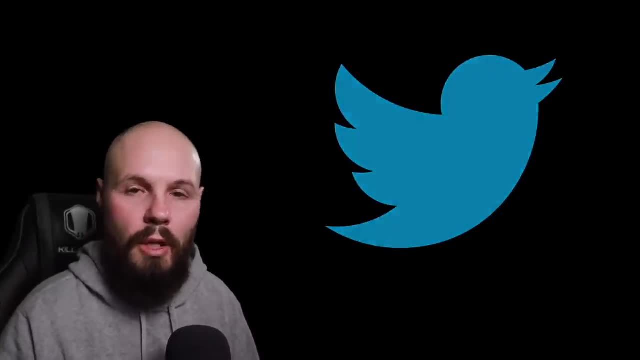 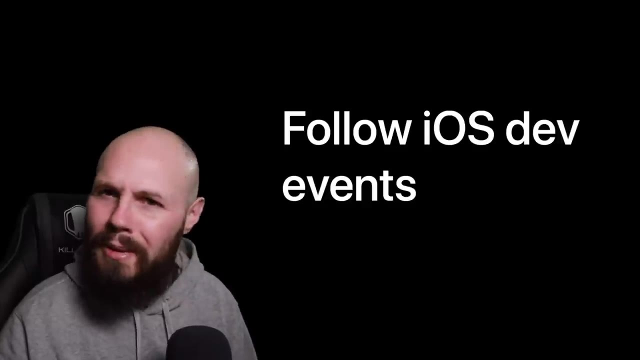 stuff to like. just prune your list So you get the good content that you want. Another great way to find followers Is to follow events. For example, WWDC 2020 is coming up in June, If the coronavirus doesn't cancel it, but that'll be an event that all iOS developers 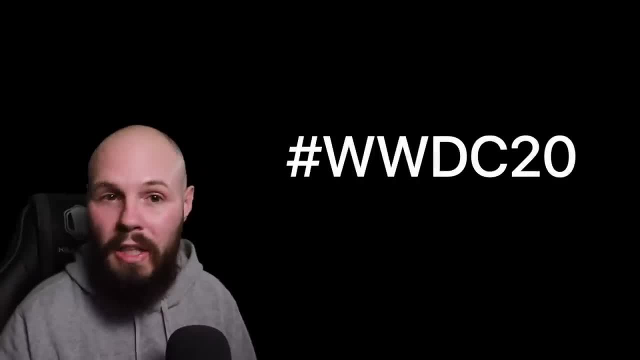 are following. They're going to be a hashtag- hashtag: WWDC 20. And if you follow that hashtag, you'll see all kinds of developers tweeting and commenting about what's going on in WWDC. That is another great way to find developers in the space. 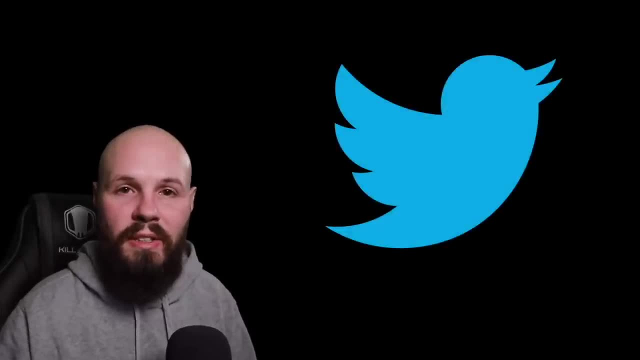 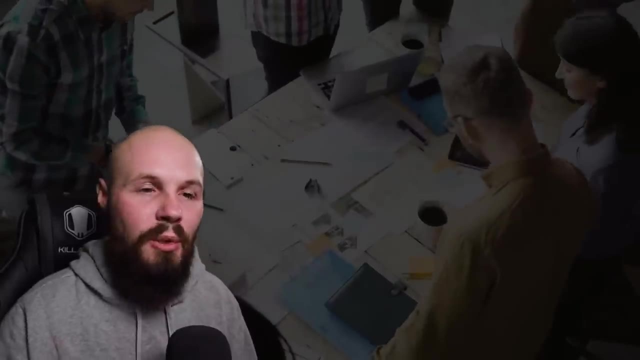 So that's some ways to find people to follow And again I'm going to have a list to get you started in the description. But again I can't stress enough: Twitter's probably the most valuable tool. It's a great way to build relationships with other developers. 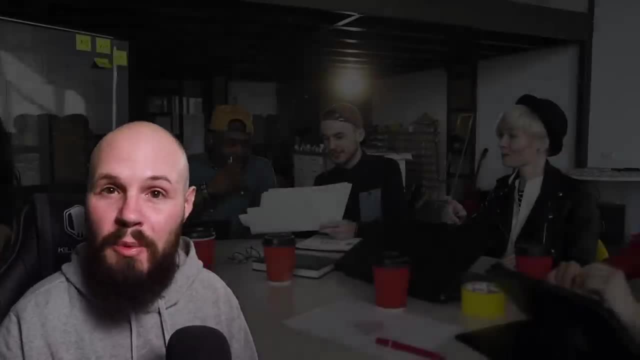 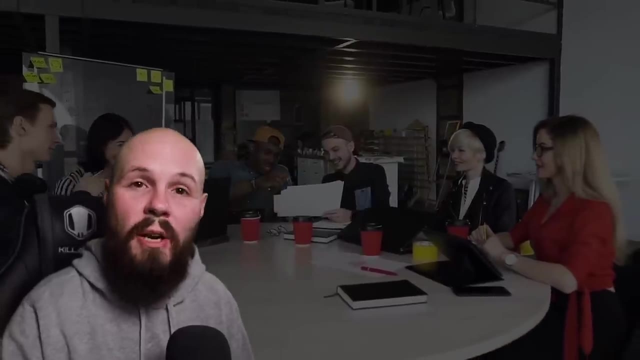 You can find help on your questions. You can potentially get jobs because you're going to know a lot of people at all the big tech companies. It's just it's so valuable and you're going to learn a lot. Again, all the content creators you know, sharing and pushing the content that they're. 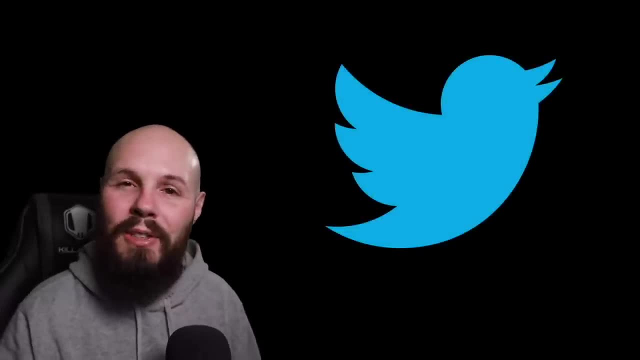 putting out there the iOS dev knowledge, So it is insanely valuable. I understand you may have reservations about joining Twitter because it does get a bad rap, but if you use it correctly because, again, you control who you follow, you control what's on your feed. 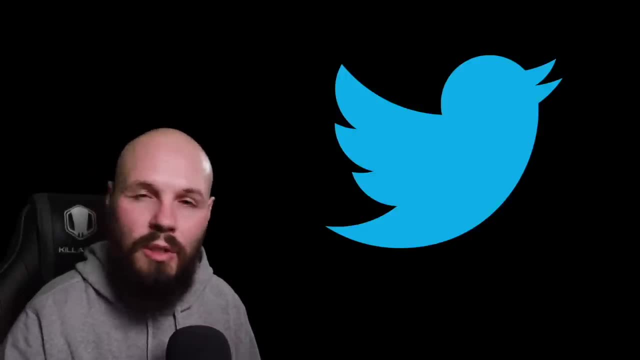 Okay, If you're constantly retweeting political stuff you don't like or bullying stuff you don't like like, just unfollow them or block them. you know whatever like. you control what you see. So if you stick to just the developer stuff, uh, Twitter is amazing. 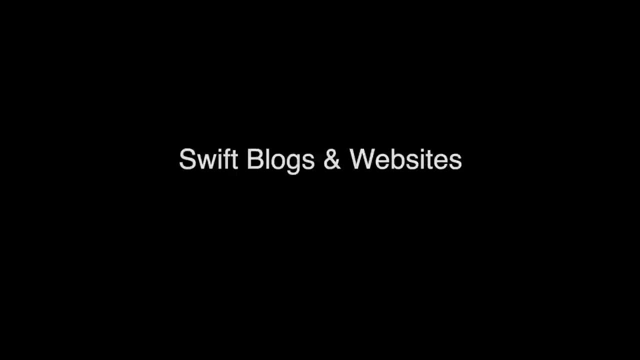 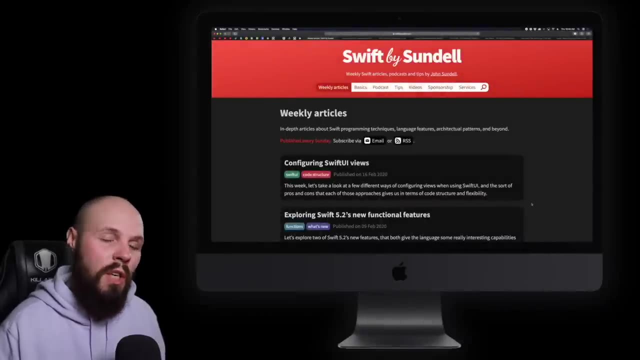 I can't recommend it enough, and then hopefully this video helped you out. The first website I want to share is Swift by Sundell, by John Sundell. Now, John is a very prominent name in the iOS Swift space, so his articles are always high. 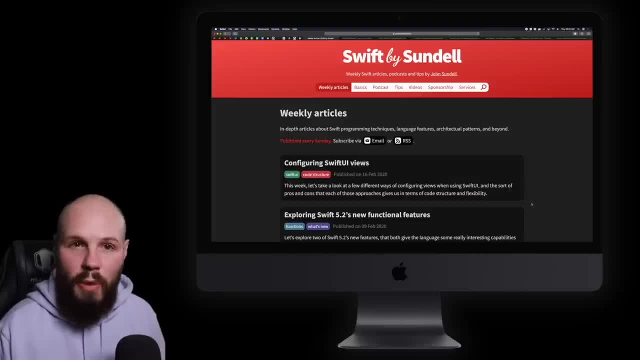 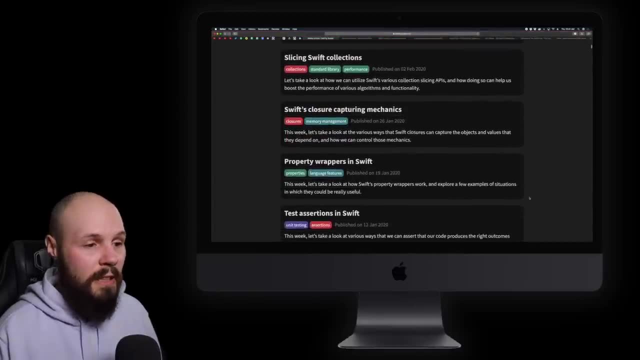 quality. Now He does his articles, and he does them weekly, by the way, usually on Sunday, uh, but some of them may be a little too advanced for the absolute beginner or somebody just beginning their journey. Those are his regular articles that come out on Sunday. 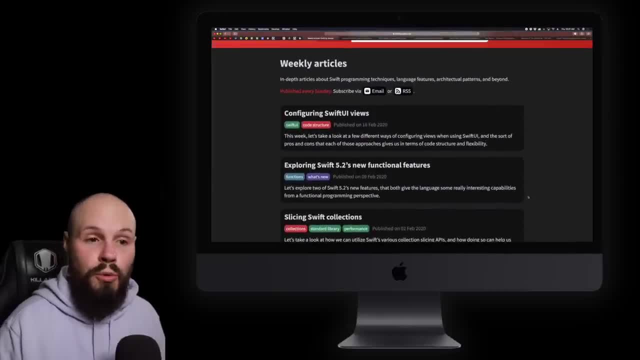 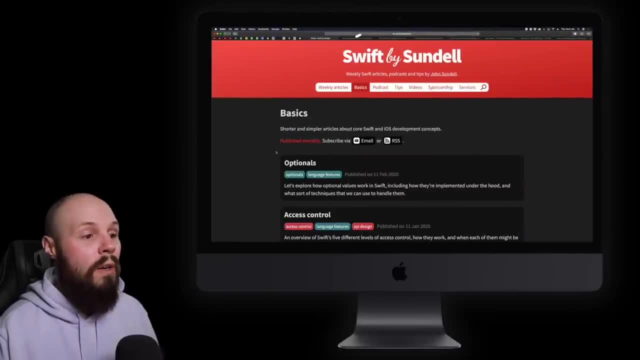 However, I still wanted to share this because one you're going to grow to, you know, look forward to these articles as you gain more experience. but he also has a basic section, as you see here, where he has again great high quality articles on some of the basic. 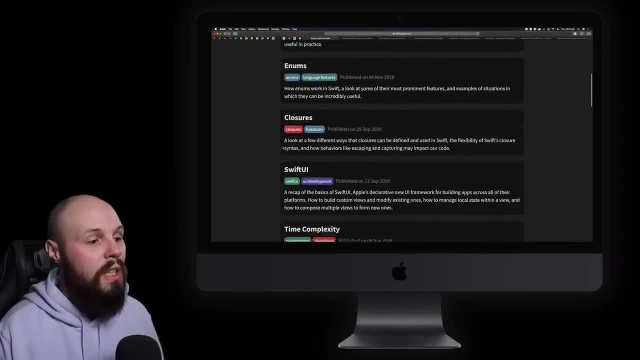 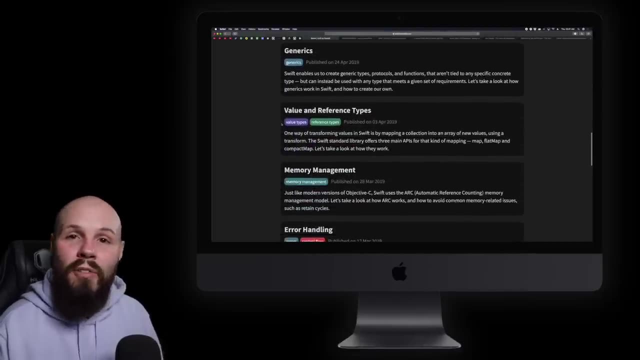 Swift and iOS developer concepts, Optionals, Enums, closures. That's always a tricky one. right Introduction to Swift UI strings, generics. So definitely check out his basics articles And then, as you gain more experience, you'll start to appreciate the weekly articles more. 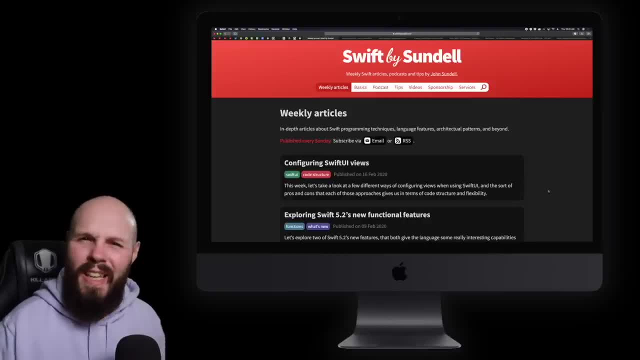 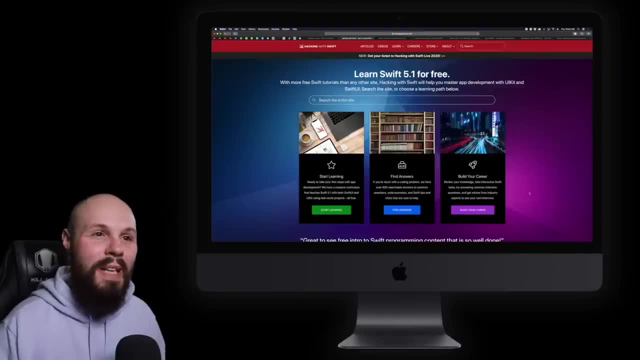 John also has a great podcast, probably one of the best in the space. Uh, we'll get to that in the podcast video, though. Next up we have hacking with Swift by Paul Hudson. If you're not familiar with Paul at two straws on Twitter, follow him. 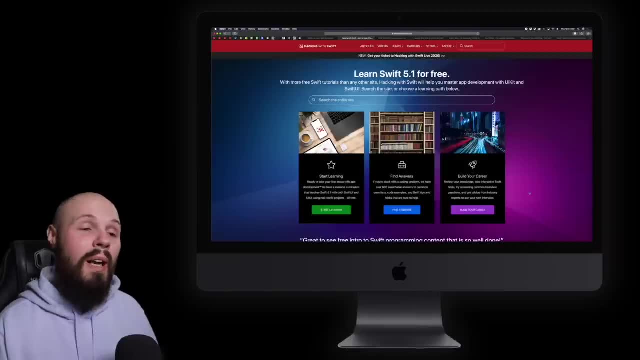 He is a content creation machine. He's got books, podcasts, articles, videos- Definitely a vital resource for the Swift community, And the great thing about Paul is that he prides himself on keeping everything absolutely up to date, right Like as soon as Swift 5.1 came out, all his articles were updated for Swift 5.1. 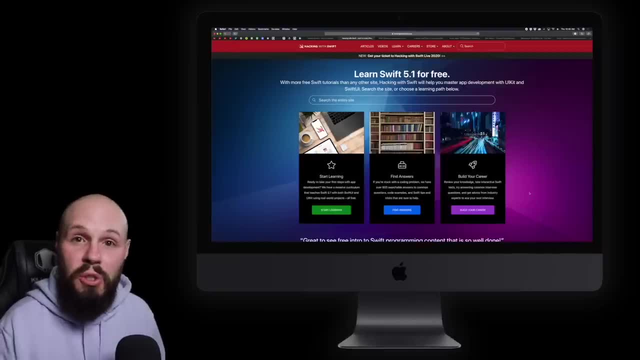 So if you're Googling and you come across a hacking- the Swift, you know solution to your problem, you can bet your bottom dollar. that is going to be the latest and greatest. It's not going to be out of date, which can be a problem. 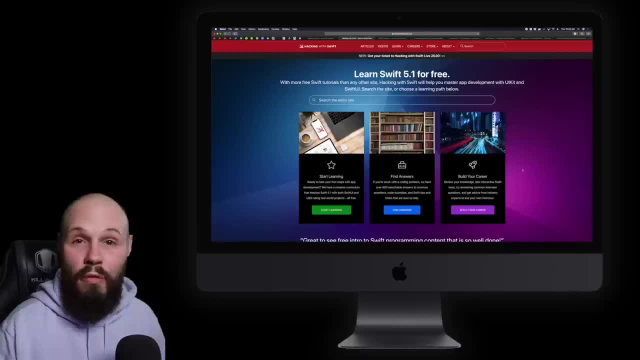 If you find something on Stack Overflow. now I can spend probably a half hour reviewing all the stuff he has on this website, but I'll leave that for you to explore. I'll share some highlights that I think are valuable for the beginners out there. 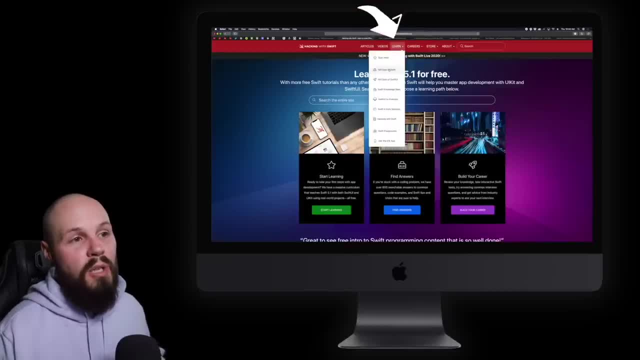 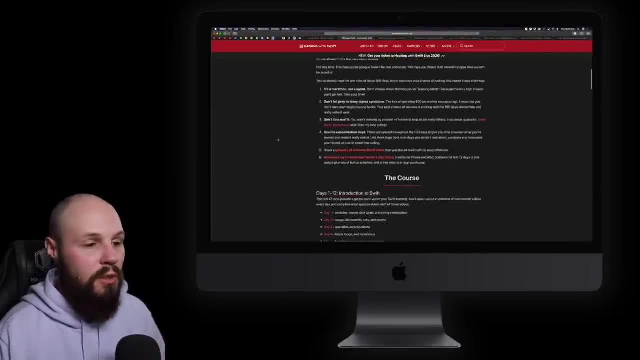 And let's go to learn tab up here at the top. And he has these two concepts: a hundred days of Swift. So this is one Swift lesson a day for a hundred days for you to continue practicing your Swift, And he goes through the rules of the course. 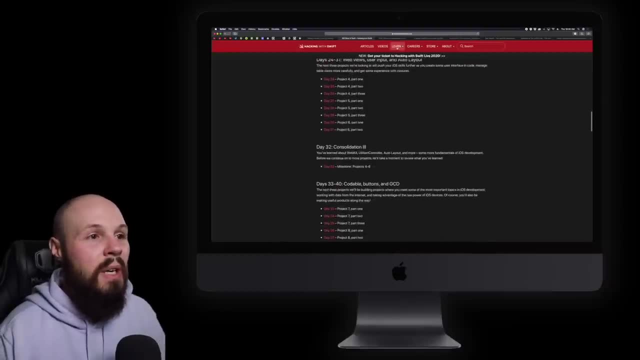 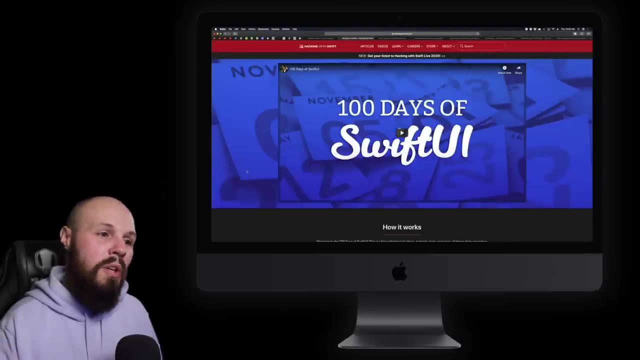 You can see the whole curriculum here. Again, I don't want to spend too much time on it, but he also has a hundred days of Swift UI. So if you want to dive into the Swift UI, same concept, one Swift UI lesson per day. 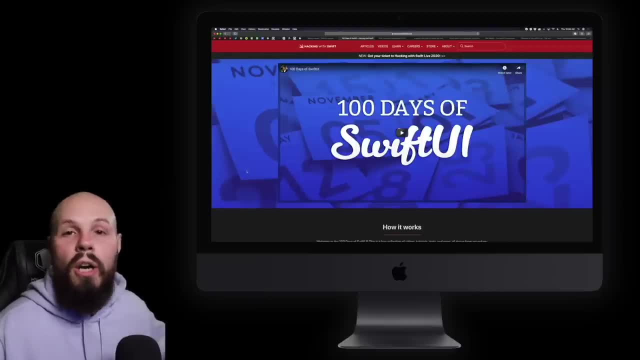 for a hundred days And there's a whole hashtag around it So you can follow along Other people doing it as well. So if you're interested in that sort of like learning, progression and practice, highly recommend this Now. admittedly, I rarely just come to the site and surf around. 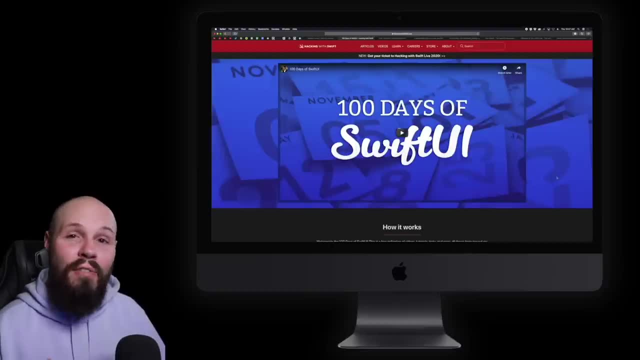 I usually get to the site via Twitter posts or most likely, and how I find the site most valuable, is a Google search. So take a common thing right: How to shuffle an array in Swift. how to shuffle an array Swift right. 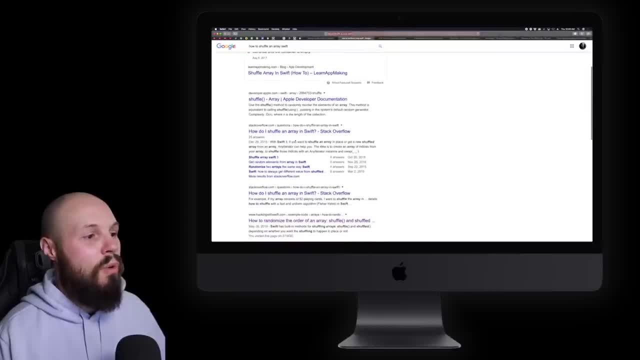 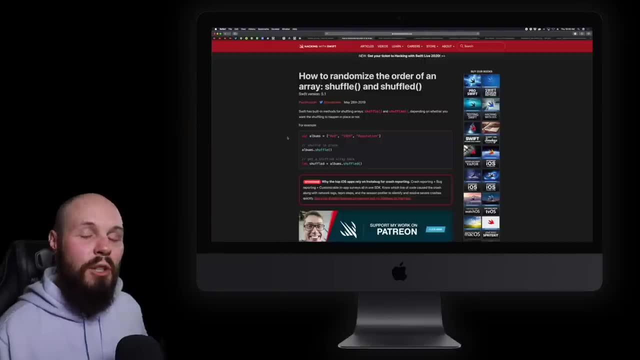 And you search for it. you know you're going to get, you know, some Stack Overflow questions, but I always look for the hacking with Swift article. You can see I already kind of clicked on this one and cause you're going to get you again, you know. 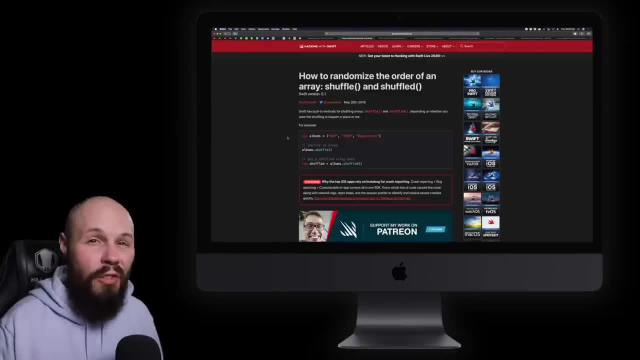 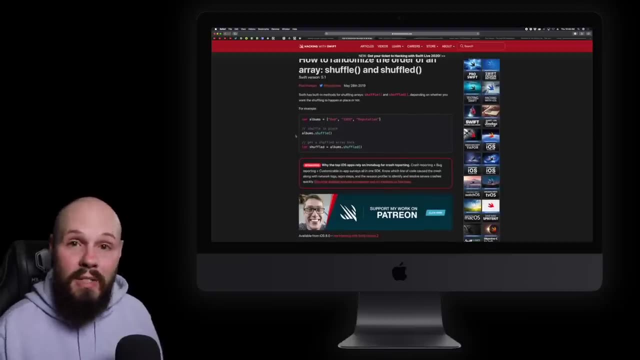 this is up to date. Like I said, a Stack Overflow article, maybe back in Swift three. it may be out of date, but you know you're going to get an up-to-date answer and it's always so concise. And this conciseness is amazing for somebody who has a couple of years of experience in 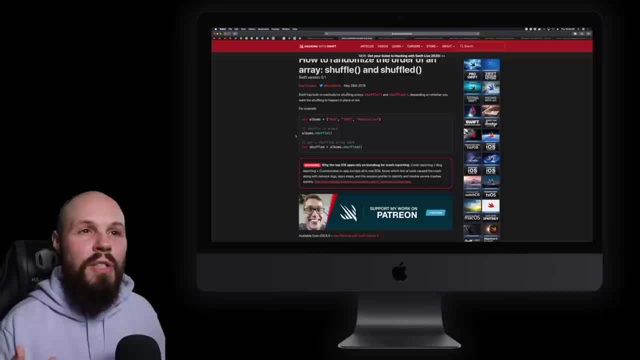 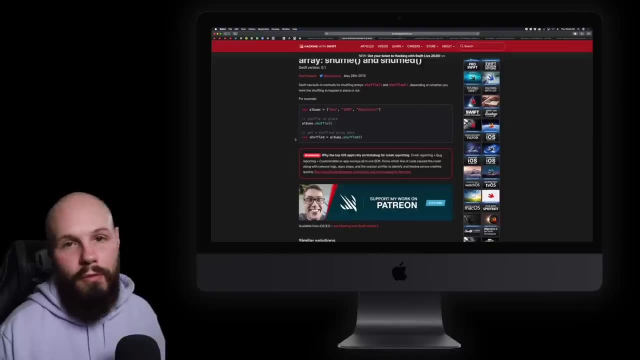 iOS development. You can just get right to the point Uh. however, if you're just a beginner, maybe you might want to look for something that gives more of an explanation. Uh, don't get me wrong, This dot shuffle and dot shuffled. very straightforward, but some of the more complex things he's. 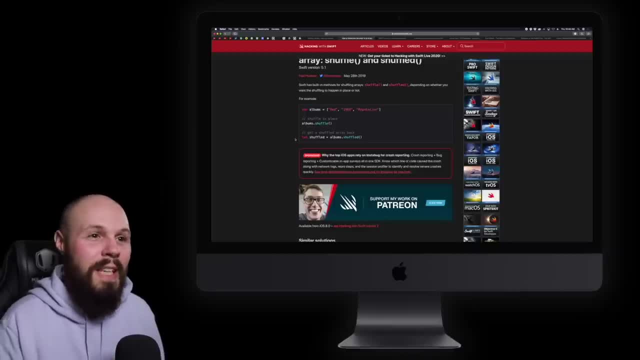 still concise, which again I love and appreciate. But if you're just beginning, I think you'll find yourself just copying and pasting to get it working. And Paul does offer- you can see all the books here on the right- He offers the content to teach you, uh, that deep learning. 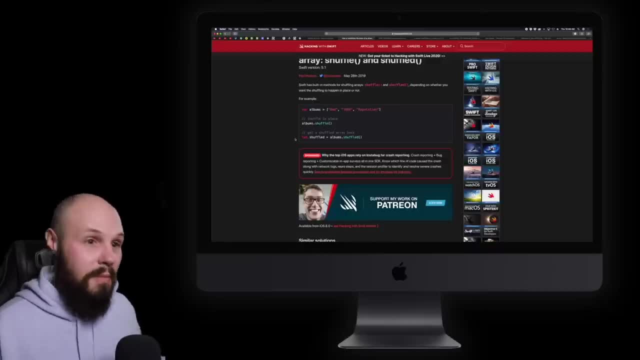 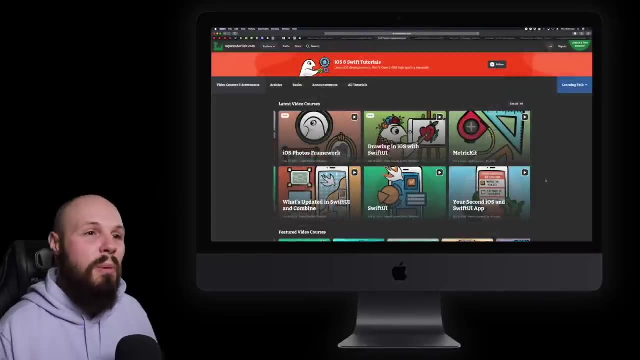 Um, but just be careful of just copy paste. It works. Okay, You know, you always want to know what your code is doing. All right, let's move on to ray wonderlickcom, another insanely valuable site for the iOS developer community. 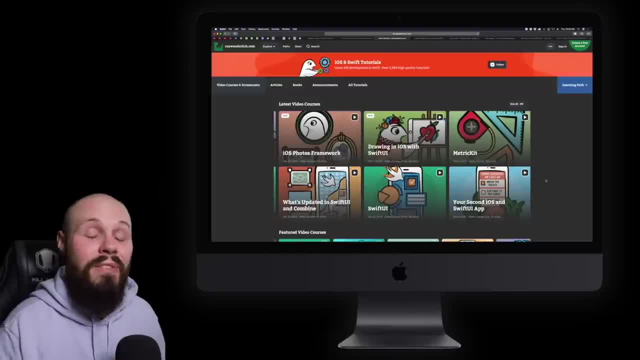 In fact, this is how I learned right back in 2015,. I pretty much lived on this site, So I personally vouch for this. This is how I learned. Of course, the site has changed a lot in the past five years, uh, but I definitely enjoyed. 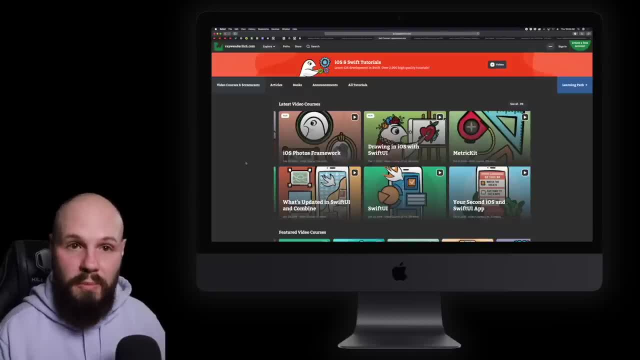 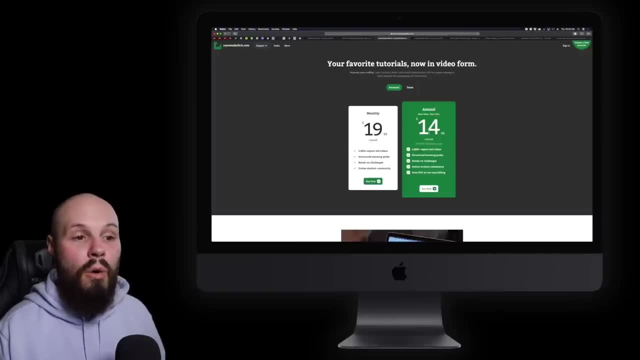 my learning on this site. Now, this site is all about videos. It is a subscription. It does cost. Let's go to the store, right? I don't want to. you know, um, find your subscription plan here. So it's either $19 a month, uh, or 1499 if you buy it annually. 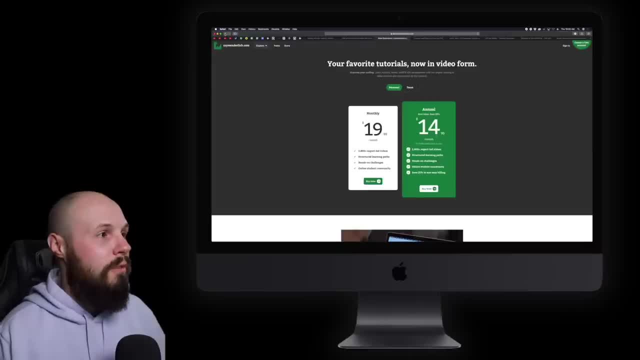 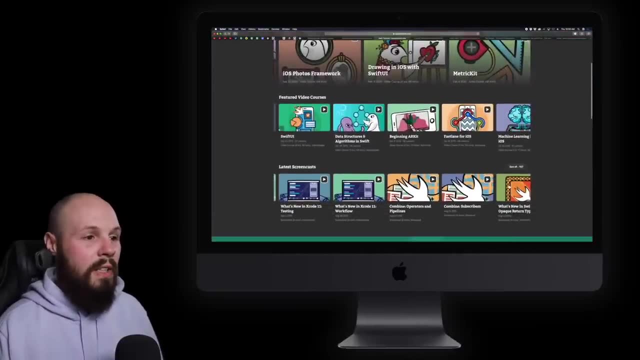 So 15 to $20 a month to invest in your iOS learning. But again, if we go back, I mean the amount of videos they have is just uh insane. on all these iOS topics, right Beginning, AR kit, Structures and algorithms, and Swift, Swift UI. 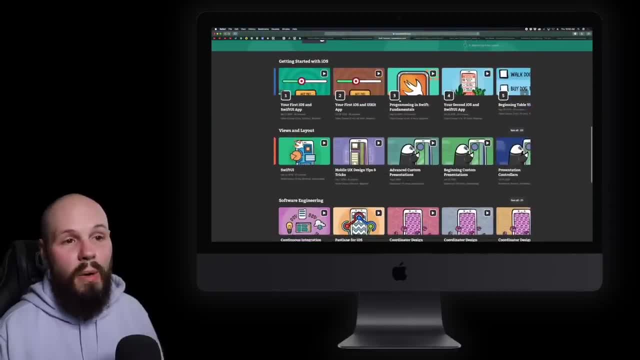 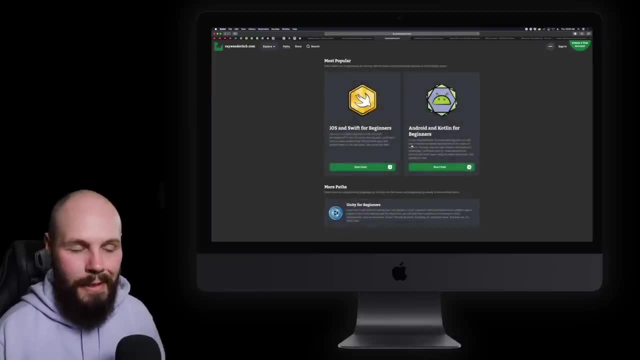 What's new in Xcode 11, the workflow and there's a whole like getting started with iOS section. So they do have a beginner and there's even if you click on paths, right. uh, we want to pick iOS and Swift for beginners, not Android and Kotlin. 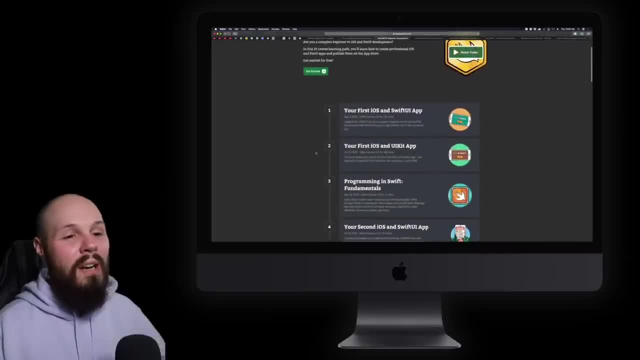 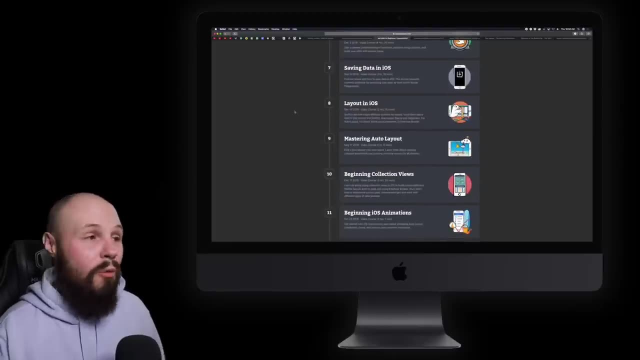 Come on, So start path And you can see there's even a nice path of courses that they have uh for you to start your iOS developer journey. you know, and continue this Now. to be honest, most of this beginner stuff we've already covered in this course, but 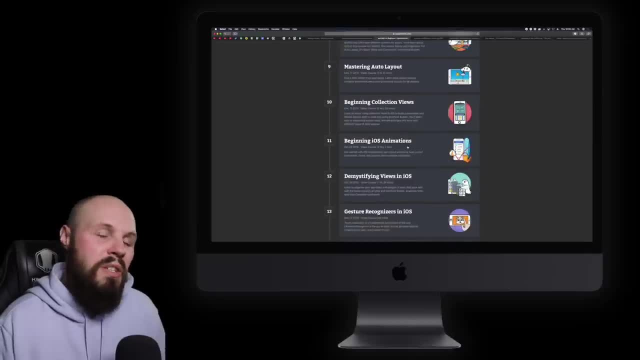 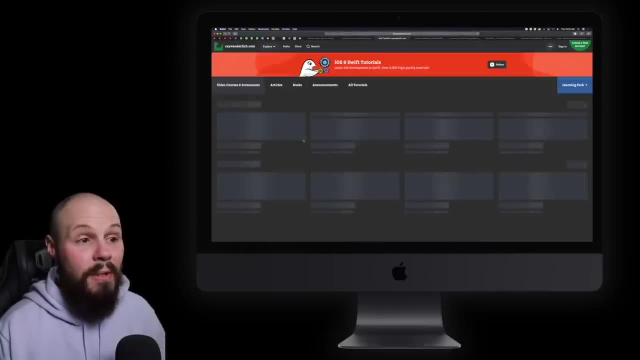 not all of it, right, You see, collection views- We didn't do that. Animations: We didn't do that. So, uh, this still can propel your learning And, like I said, that's just their beginner path. but even after you're not a beginner. 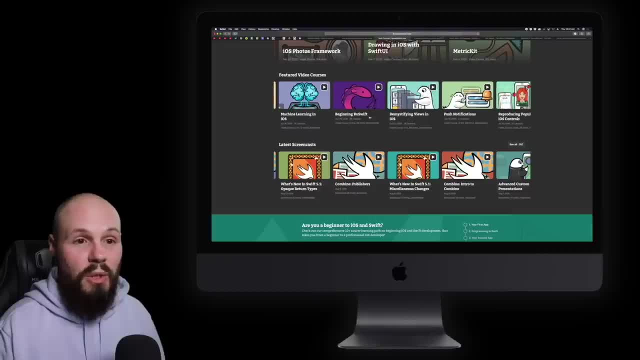 anymore and you know you want to learn some like advanced topics, like machine learning for iOS, as you see here. push notifications- just an insane resource. again, yes, it is $20 a month, or 15 if you buy the annual, but in my opinion that's a small investment into. 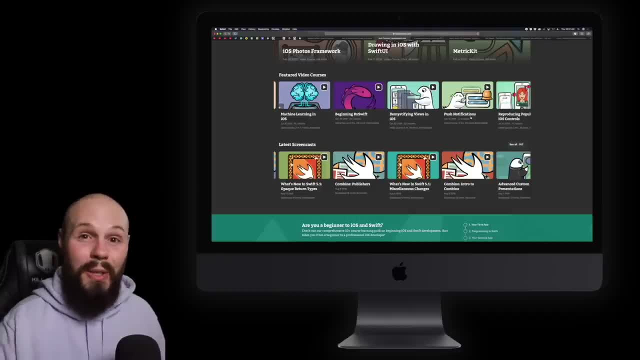 your learning to make this a career. And again, this is how I learned. I spent that 20 bucks a month for about a year and just lived on this site, So I enjoyed it Moving on. This next one is by Antoine Vander Lee. 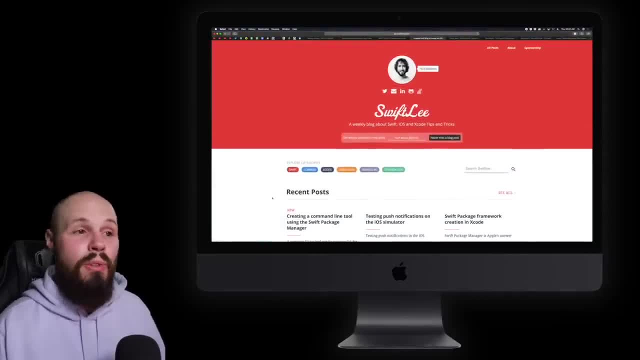 Uh, he just posts a lot of basically all skill levels, from beginner to advanced, So he's also a good follow on Twitter. Give them a follow. That's how I discover his articles He puts it out on Twitter. I always check them out. 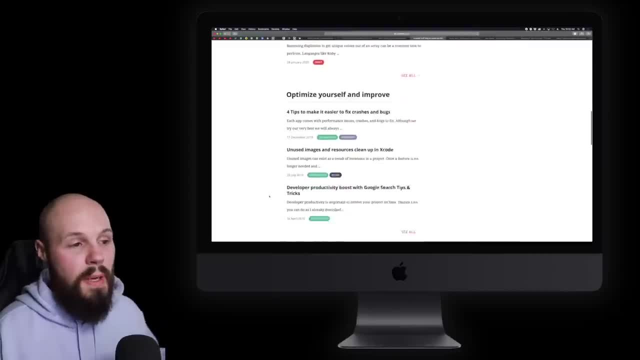 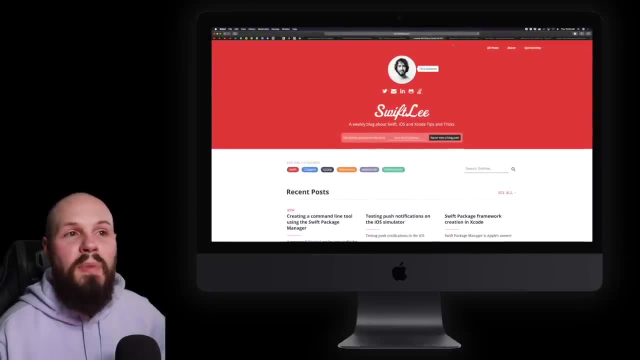 Uh, you're definitely gonna learn a lot with his articles. Um, I could scroll here, but it's basically just a myriad of topics again, all the way from beginner to advanced. but definitely a must follow in a, definitely a must bookmark. 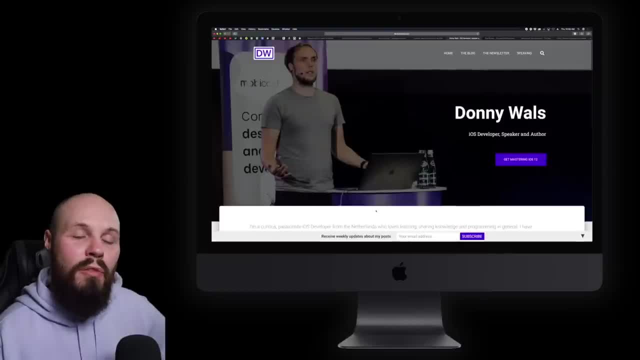 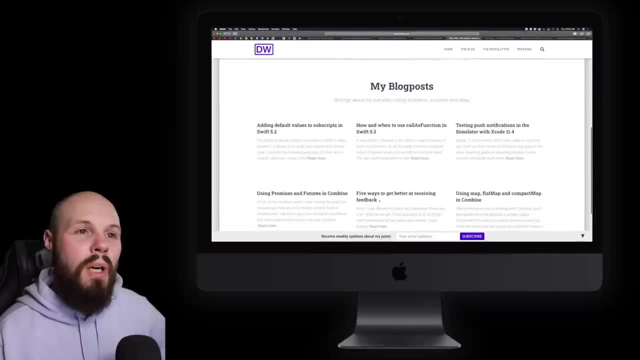 Same thing with Donnie Walls here, a relative newcomer on the scene, if you will. probably for the past year he's been putting out content, but he's a. he's an iOS developer at Disney and he again same thing, kind of similar to, uh, Antoine Vander Lee- not, not that they. 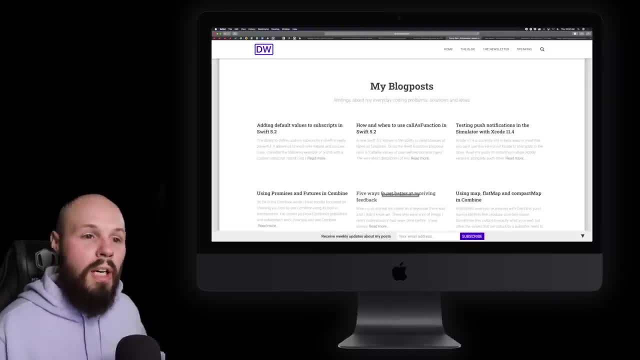 put out the same content, but he posts a variety of beginner uh to advanced stuff. But if we go to the blog you can see some of the topics you know. uh, these are probably more advanced stuff than you're looking for. 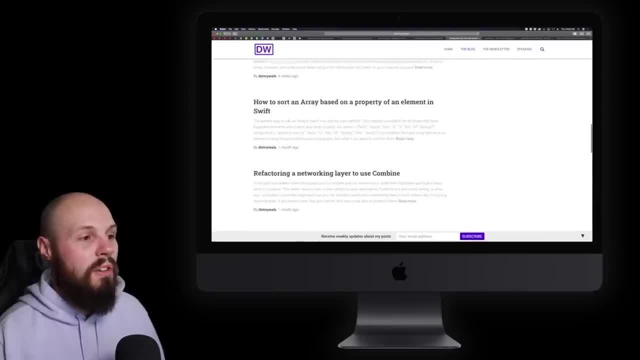 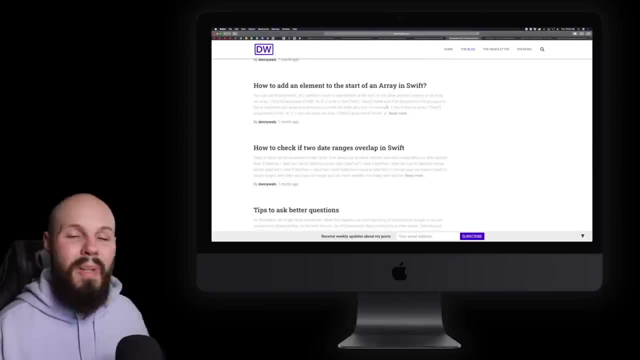 But back down here you can see some relatively uh, simple stuff for like how to sort an array based on a property, how to add an element to the start of an array. So he does do some beginner stuff, but again, a lot of these resources that I'm showing 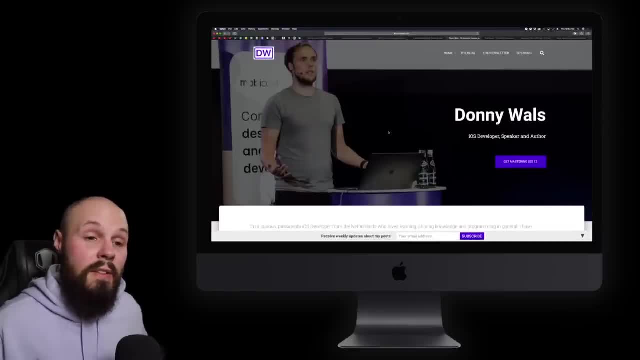 you aren't necessarily just beginner resources, right? Instead, this is the stuff that I use and learn to this day, So you may have to grow into these resources a little bit, but you're definitely going to want to follow them. Next up, let's talk about iOS dev weekly by Dave Verwer. 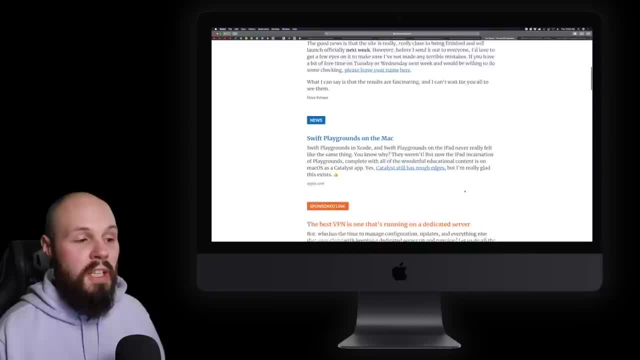 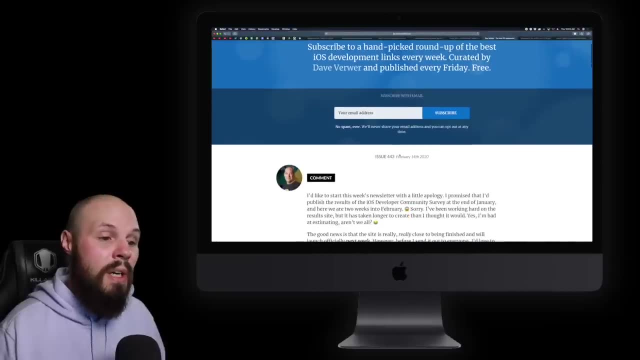 So iOS dev weekly is a newsletter. However, you can come to the website here and see the newsletter. He shares a bunch of great links that comes out every Friday. I recommend signing up for the newsletter so it gets delivered right to your email. 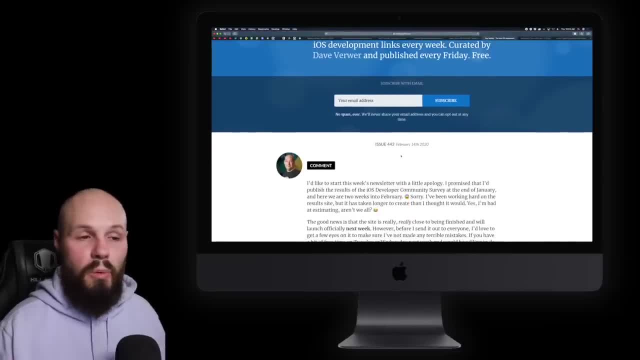 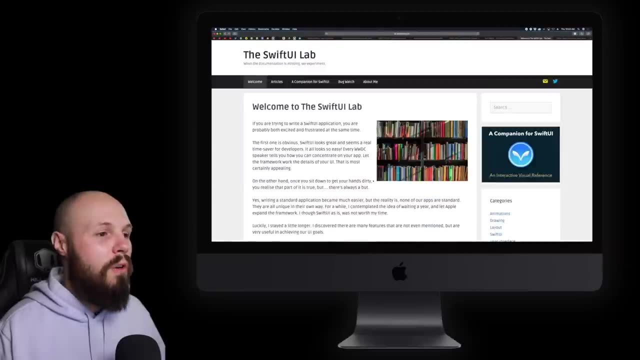 This is the premier newsletter, uh, in iOS developer world. Like, if you're an iOS developer, you got to subscribe to this newsletter. Like, just enough said and let's finish up with some Swift UI focused stuff. I remember, like I said, the bulk of this course does focus on UI kit, but I still want. 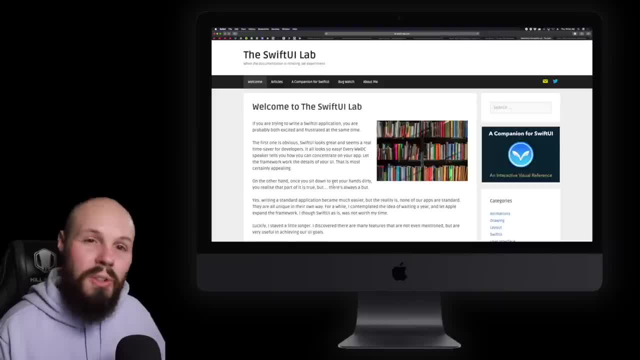 to expose you to Swift UI. uh, even though it's still super early in Swift UI- I can't emphasize that enough- but there are some blogs and websites that are popping up that are dedicated to Swift UI. One, for example, here is the Swift UI lab. uh, and let's go to articles here. 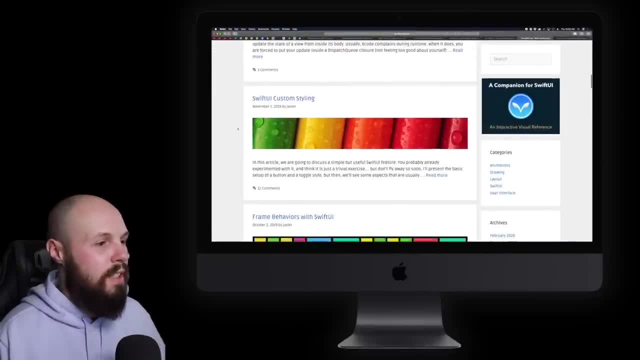 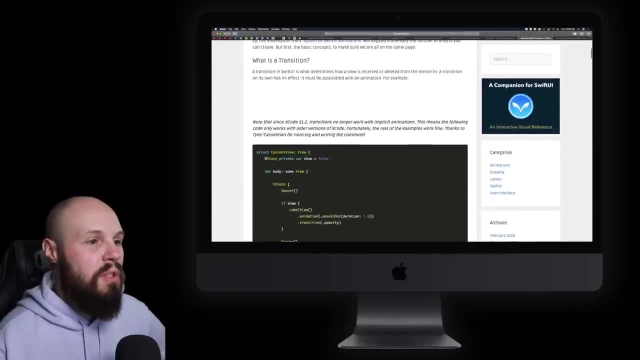 And I like these articles cause they're very visual. We'll scroll down to one that I checked out here a little bit ago just to make sure. So like advanced Swift UI transitions. right Yeah, So this is the topic of Swift UI transitions, but you can see his articles also have like: 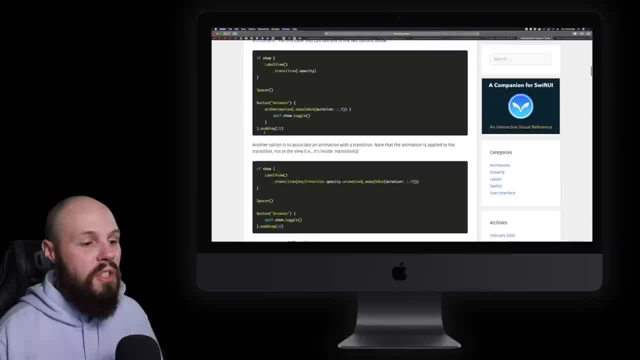 animated gifts to show you what you're building. So you can see this is transitioning. It looks like a button here all the different transitions. I'll let the screen play. You can see sliding to the right: fading in, fading out. 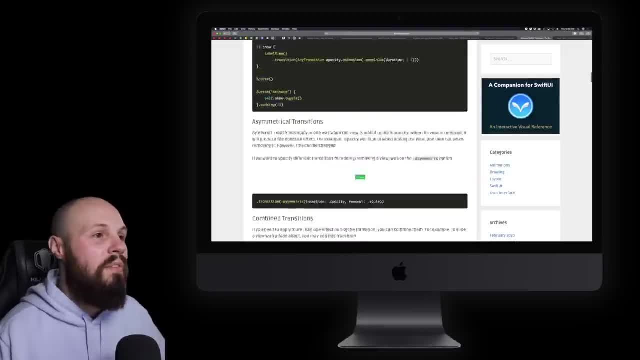 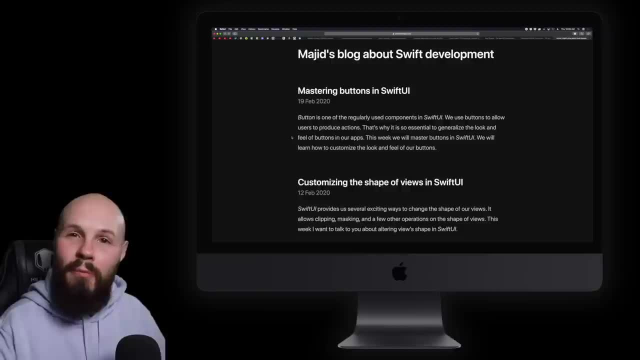 So their articles are very visual, which is what I like about it. So definitely, if you want to dive more into Swift UI, bookmark the Swift UI lab, And then also you have Majeed's blog here. to finish up here, much more simple looking. 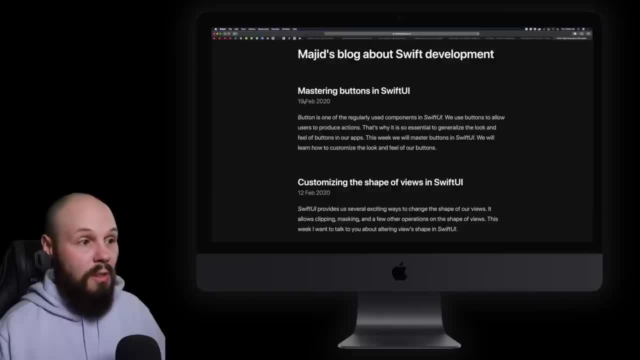 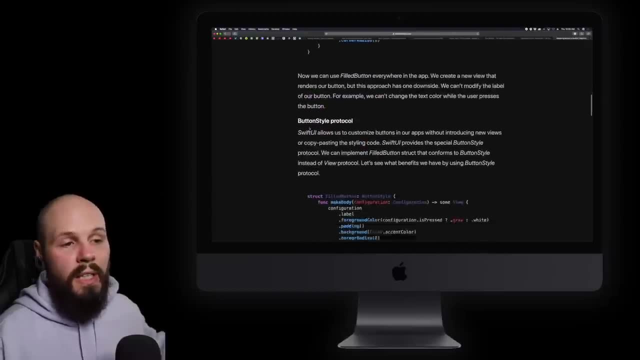 but this is also super dedicated to Swift UI. Uh, for example, just the latest one, on February 19th, mastering buttons in Swift UI. Click on that. This is basically just how to use buttons in Swift UI And, again, very visual, showing you what you're building. 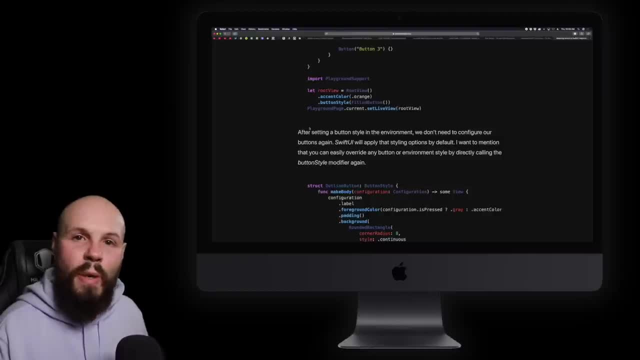 So big fan of that. That wraps up the blogs and websites that I visit on a regular basis to continue my learning and that I think you should bookmark. Of course there are a ton more websites out there. I'm not saying this is like the only list. 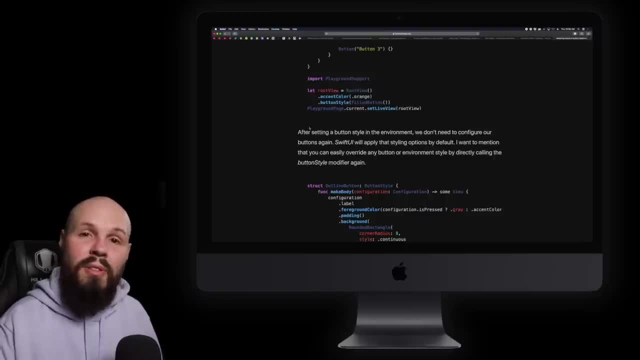 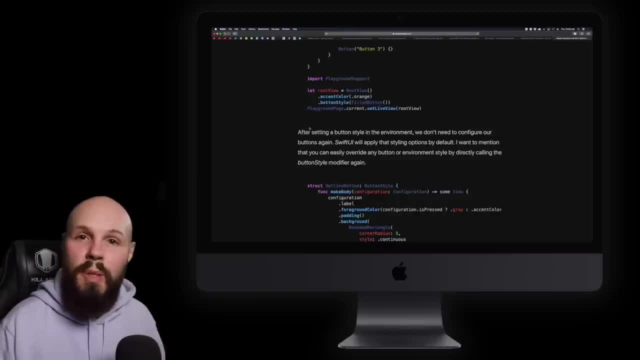 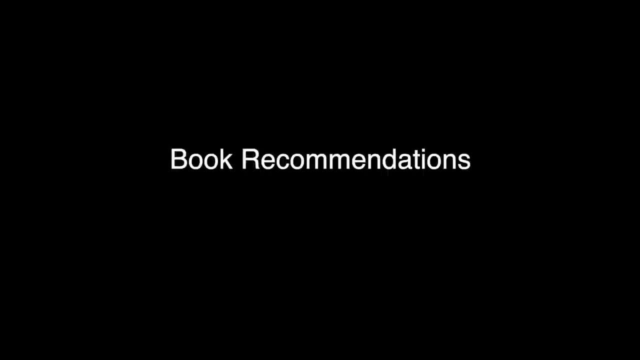 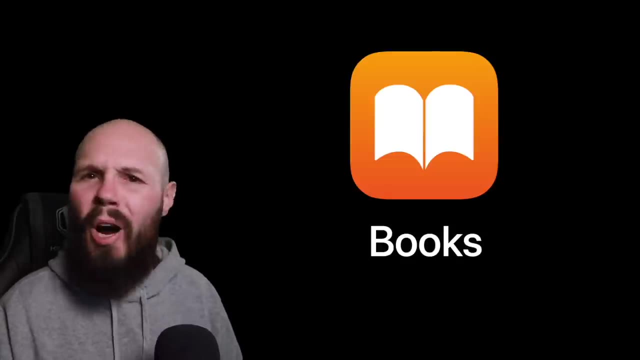 the next video. In this video, I'm going to give you a bunch of book recommendations for you to continue on your learning. uh, two quick disclaimers. It's impossible for me to cover every possible book out there, So if you have a great book that you really liked that I didn't list, please leave it. 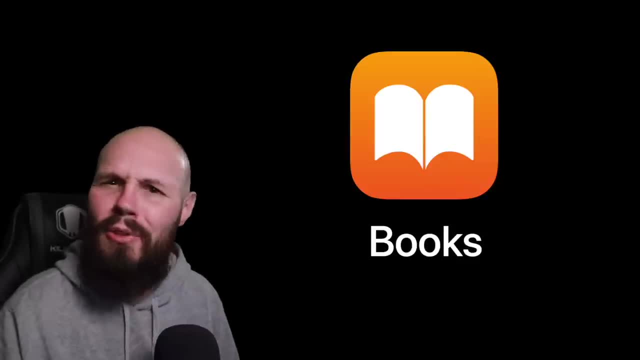 in the comments. And again, if you're watching this video, make sure you check out the comments for further suggestions. I'm going to leave links to all these in the description of the video, but I want to be completely transparent. A lot of them will be affiliate links and that's just because, like I, have relationships. 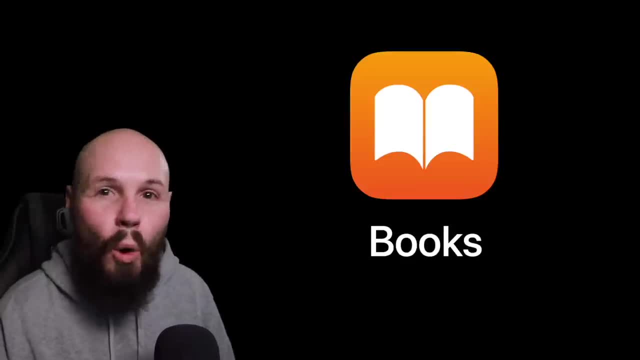 with, like everybody in the space. So I'm not trying to point you only to my affiliate links. That's not it at all. If you ask 10 developers, they're probably going to give you a list very similar to mine, but I do want to be upfront and honest about that. 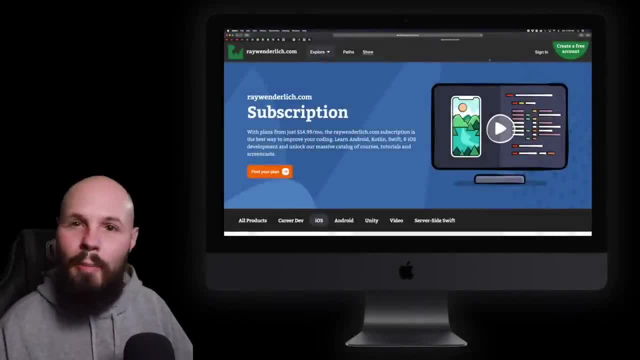 All right onto my recommendations. First up is the site that I use the most to learn back in 2015, when I was getting started, And that is raywonderlickcom. Now we're going to scroll down. This is the video subscription service. 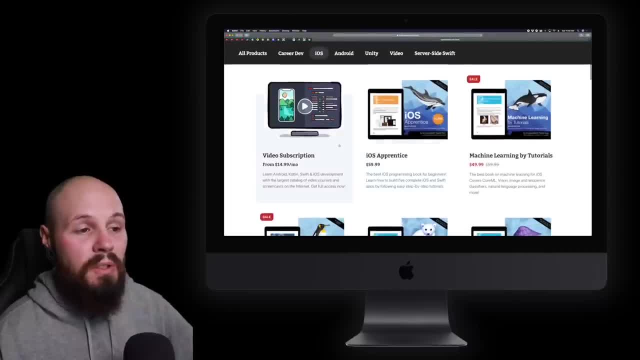 You can do that if you like, But we're talking about Ray Wunderlich, We're talking about books here, Right? So I'm going to slowly scroll down. You can see: iOS apprentice teaches you everything. just about iOS, essentially. You see machine learning, mastering Git. 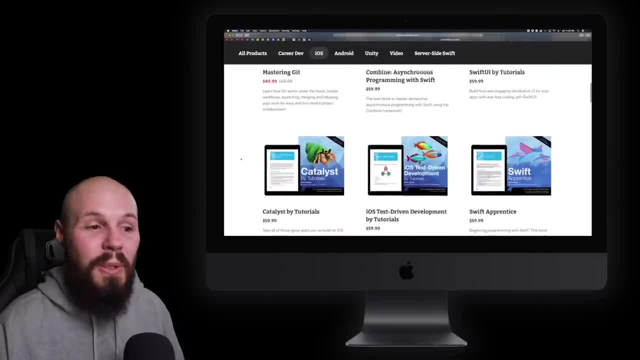 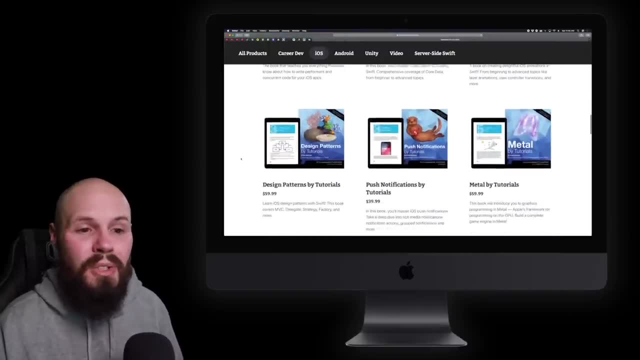 I'm not going to list all of them. The point is, as I scroll I'll talk. You can see there are a ton of topics. So he's got like 50 different books on everything: animations, core data, push notifications. 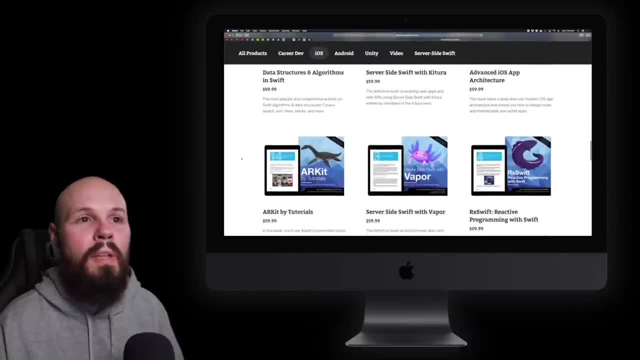 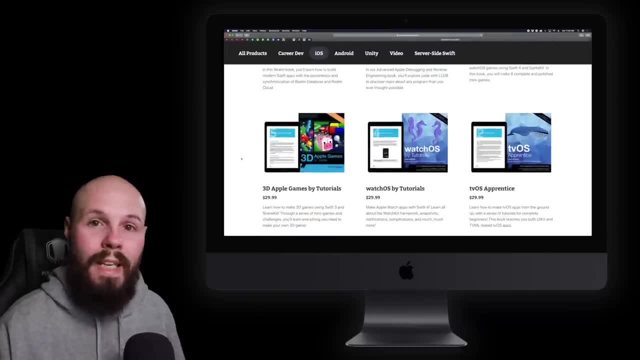 right, There's just the list is so long. So Ray Wunderlich has a very vast library for pretty much any topic you may want to tackle in the iOS development space. And again, Ray Wunderlich is how I got my start. 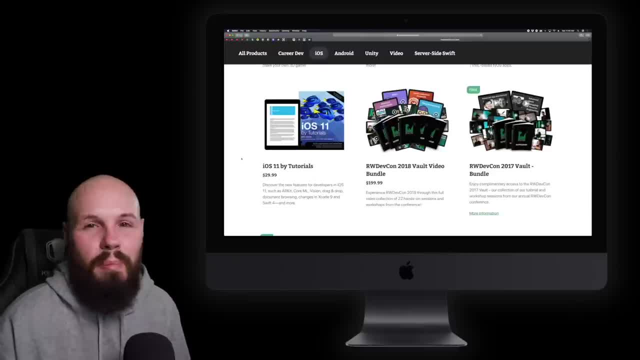 So I can kind of personally vouch for you know the quality and it is. it is one of the biggest names in the space, So definitely check it out If you're interested. Next up we have hacking with Swift by Paul Hudson. 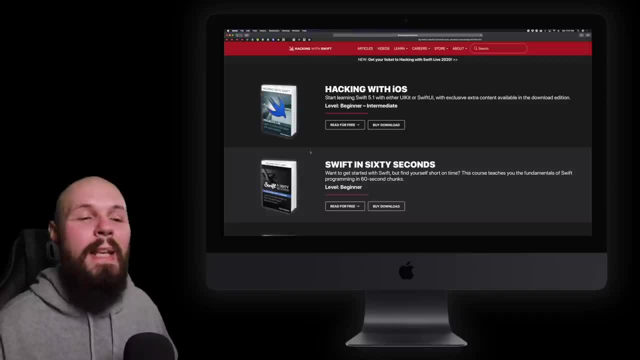 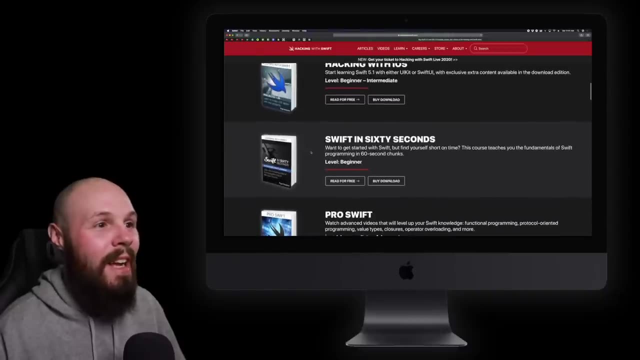 You may start to see these names repeat a lot because, again, there's a lot of big names in the space that create a ton of content. but, very similar to Ray Wunderlich, Paul has a book on almost every topic, right Hacking with iOS, just the basics. iOS Swift in 60 seconds- pro Swift design patterns. 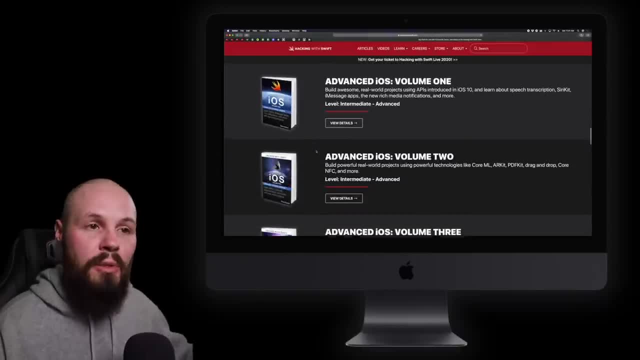 testing Swift UI. right, Again, I'm not going to like list everything, I'm just going to scroll down. I'm not going to read everything, but you can scroll down and see all the books here And I think, really, at the end of the day, right. 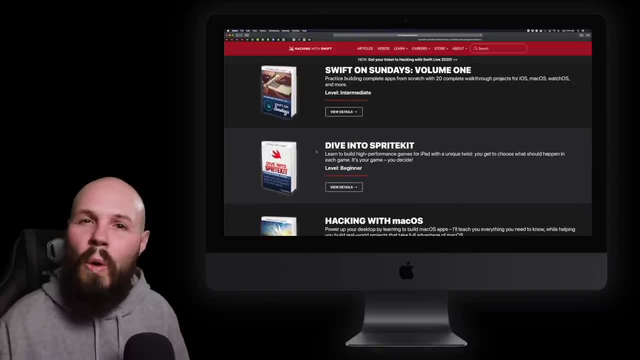 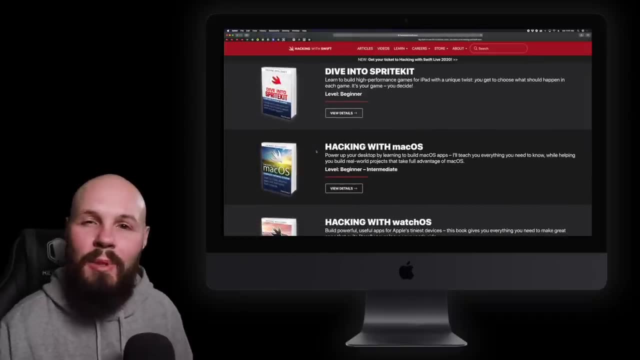 Like there's a lot of great teachers out there, but what teaching style, what writing style resonates with you the most? That's whose books you should go to. So again, I know I'm kind of showing a lot of the same topics, but again you're going. 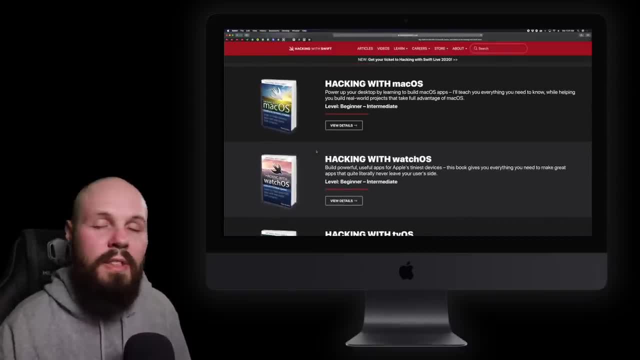 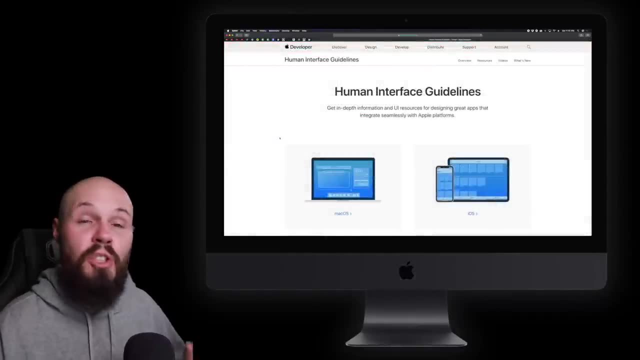 to see different teaching styles and you may resonate more with different teaching styles. Next up, we have the human interface guidelines. Now, this isn't like a Swift tutorial book, like Ray Wunderlich or hacking with Swift, but this is directly from Apple. 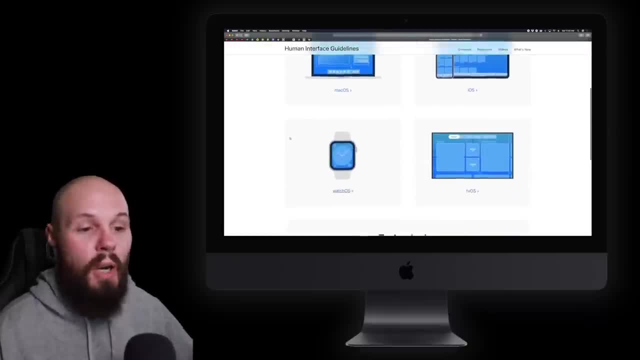 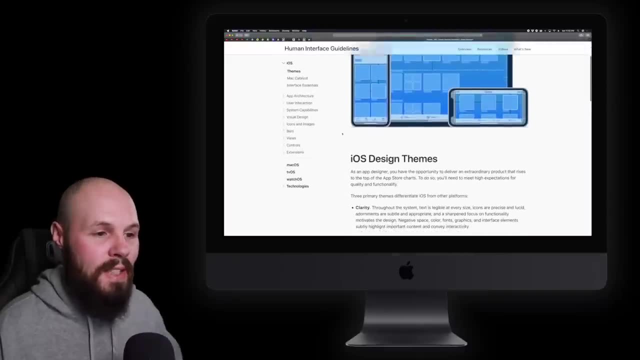 Basically telling you the best practices for their platforms. Like you have Mac OS, watch OS, TV OS, Let's click into iOS to show you some things here. So it's basically going to tell you how to properly design and use best practices in. 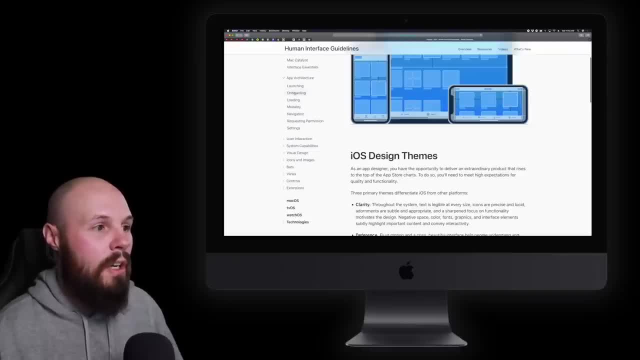 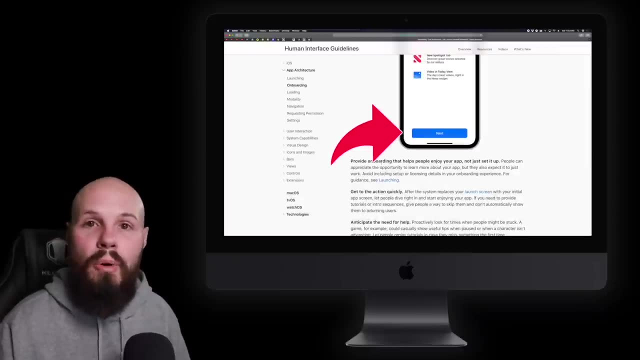 your app. So over here on the left you can see we have like app architecture, onboarding, like how that should work, And it's going to tell you again the best practices, Like, for example, this blue button here, like it'll tell you every touch target should be. 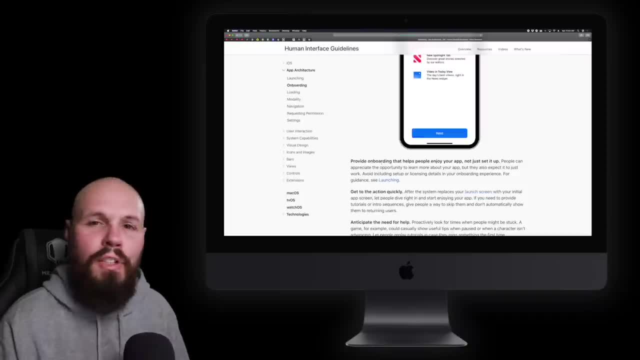 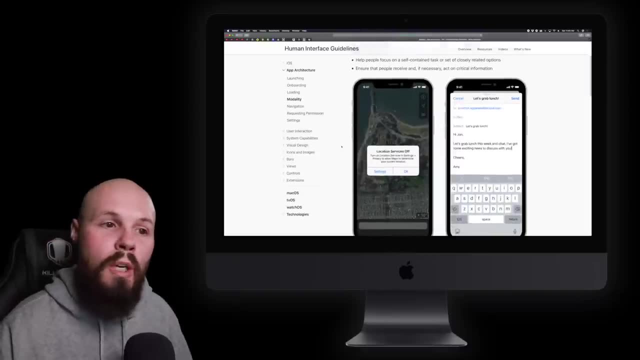 at least 44 points tall, because again, that's the size of the average human fingertip. right, It's stuff like that. right A modality right. It'll tell you how to properly create your modal sheets coming up. 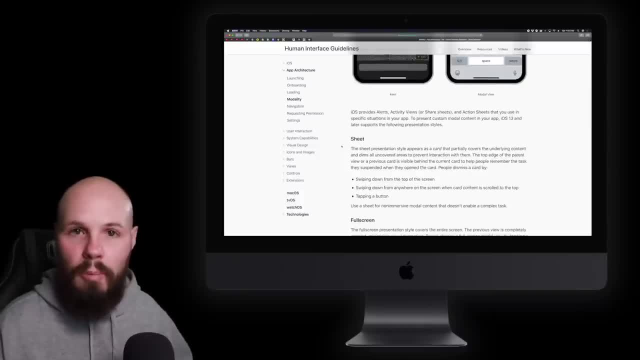 So I think this is just a must read for all iOS developers, because it's going to tell you all the best practices on building iOS apps straight from Apple, And again more things. let's go to the user interaction section, right Drag and drop. 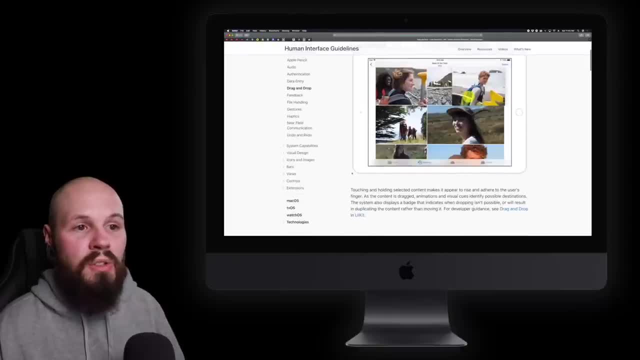 You know it'll tell you again the best practices on using drag and drop. It'll usually have videos to show you- you know- how to do it. I mean it's not going to show you like a tutorial on how to do it, but it's going to. 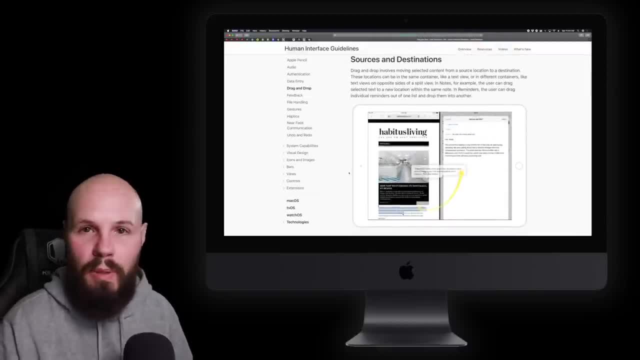 show you the best practices on how to implement it. Okay, How to implement it on the iOS platform, right? That way, your iOS app feels like an iOS app and not some just random concoction you came up with. And the reason that's important is because iOS users expect a certain you know way. 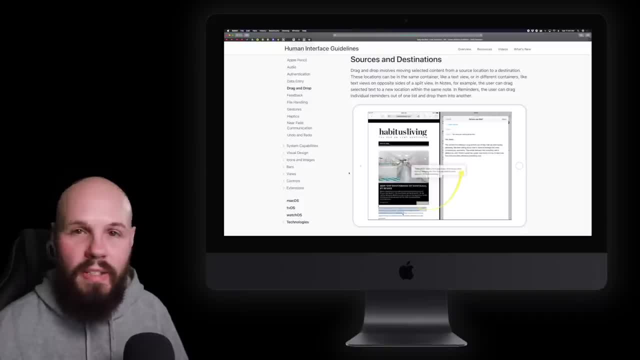 of doing things, And if every single app on iOS had all kinds of different navigation, all different ways of doing things, like it would be a bad user experience, right? But when users use an iOS app, they kind of intuitively already know how to use it based. 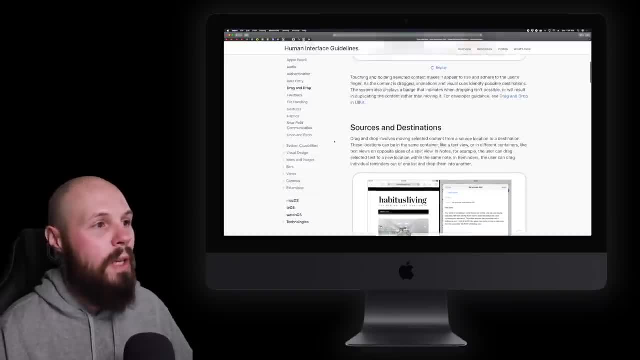 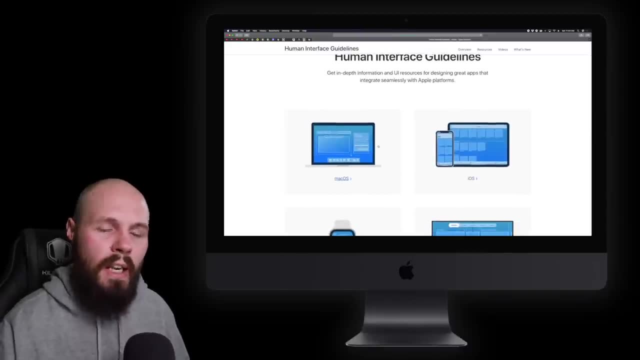 on the best practices Apple has set forward. So if you want to learn more about those best practices Again, Human interface guidelines: they update it constantly. For example, they just came out with a new update all about you know Siri and how to. 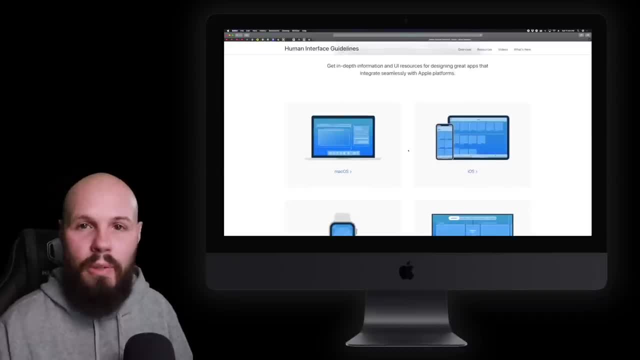 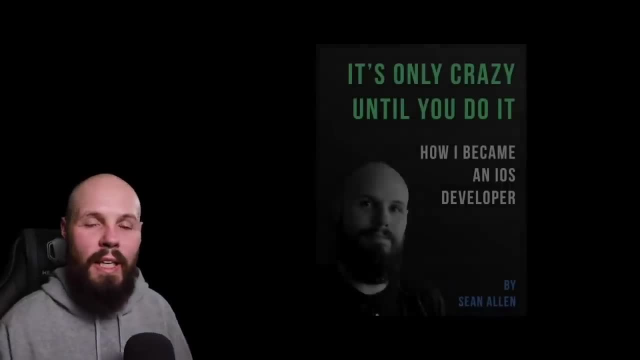 implement that, So it's always updated. I always recommend iOS developers read through this at least once a year. Anyway, it's great stuff. It's a must read. Next up, we have a little bit of a shameless plug, and that is my own book called it's only. 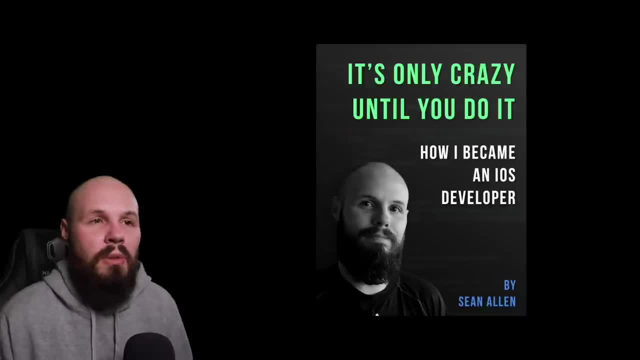 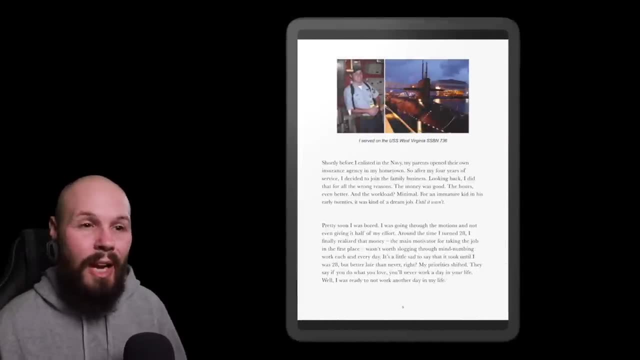 crazy until you do it, How I became an iOS developer. And it tells my story, because my story isn't the normal path, right? I went into the Navy right after high school. I was an insurance agent for six years. I went back to school at 30.. 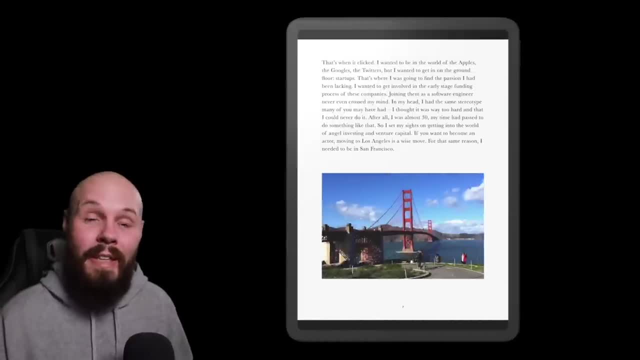 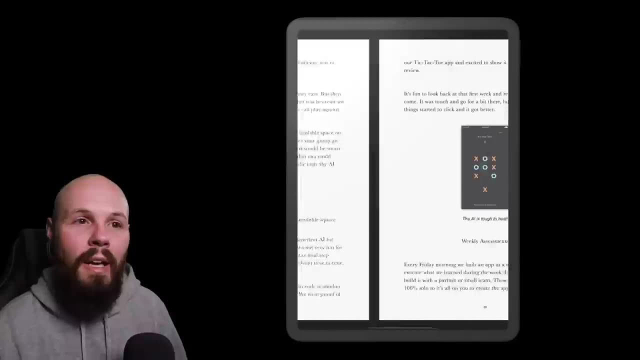 Like I didn't really know what I wanted to do in my twenties And then I wrote my first line of code at 32 and just kind of fell in love with development. And it tells the story how that happened, how I learned to code, how I ended up getting 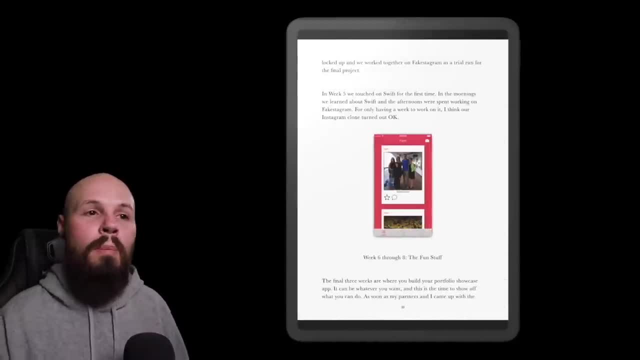 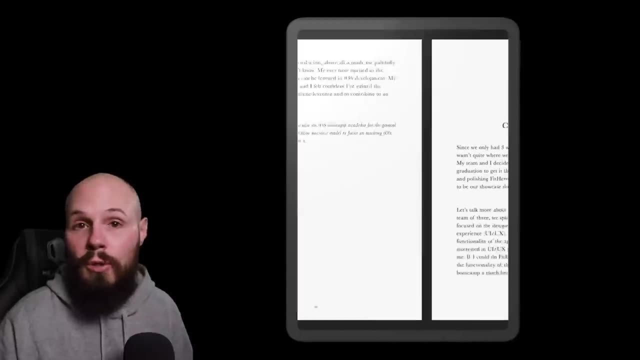 my first job and basically how I launched my career, And my goal for the book was for people exactly in your spot that are just learning to kind of be inspirational, right, Because, you know, maybe some of you out there are a little older, maybe you're not the 22- 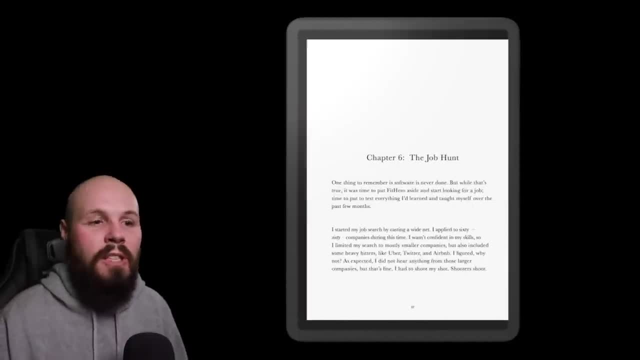 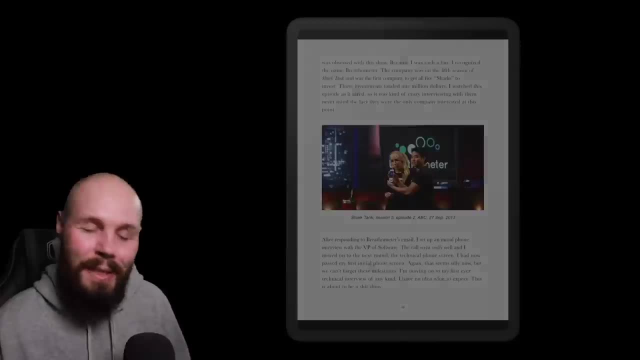 year old kid, right. So hopefully it'll be inspirational to you to just tell you my story And again, it's only like 60 pages, short little ebook that you can probably knock out in a couple of days but I've been told is very inspirational. 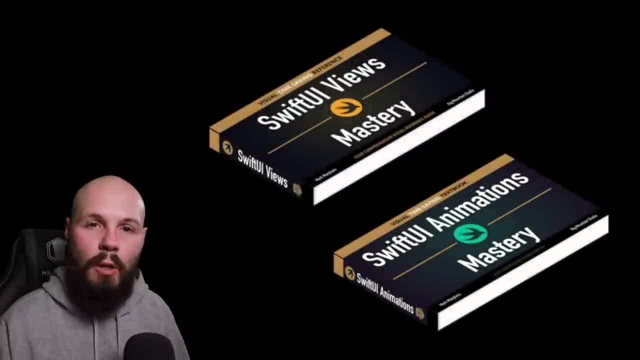 And that was my goal. Next up, if you want to dive into SwiftUI, we have some book by Mark Moikens, another YouTuber. He's created two SwiftUI books called SwiftUI Views Mastery and then SwiftUI Animations- Both of these. what I like about them is they're extremely visual. 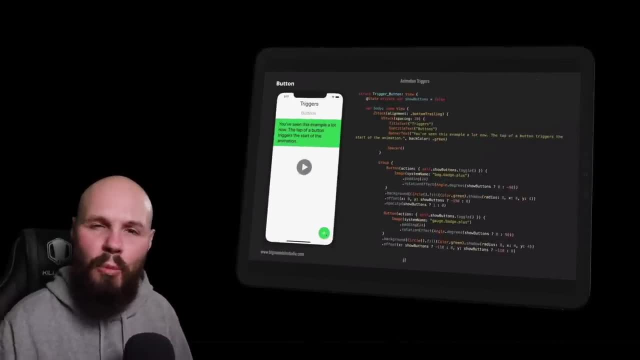 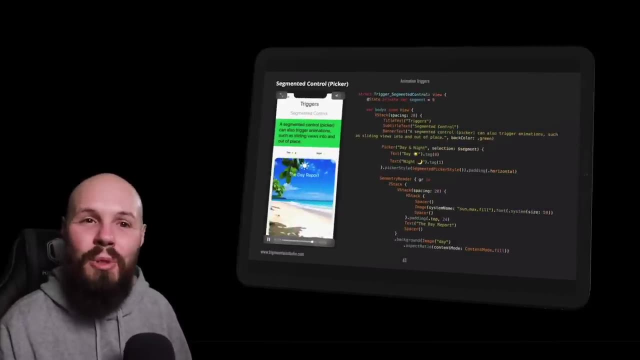 And I'm actually diving into SwiftUI myself, building a couple apps in it, really starting to learn it, And I've been using Mark's book myself And, like I said, they're page turners. I call it Because they're so visual. I always want to turn the page because I want to see what's. 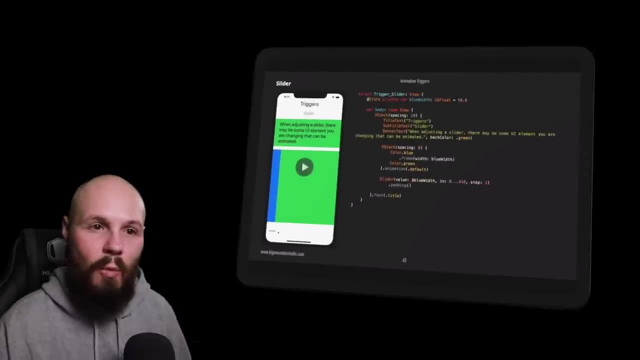 on the next page And you're not. it's not like a typical book, as you can see here, where you just have to read paragraphs and paragraphs. It's really I don't know. it's really short, quick, bite sized stuff. 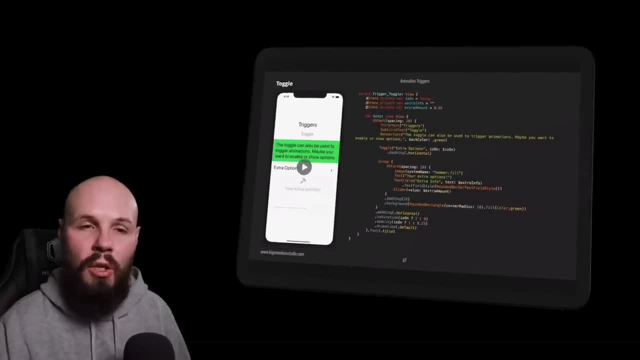 And that's what I like about it. And then again the visuals to actually show you what the code is doing. It's great stuff. So you know, of course, you know Ray Wunderlich Hacking with Swift. they all had books as. 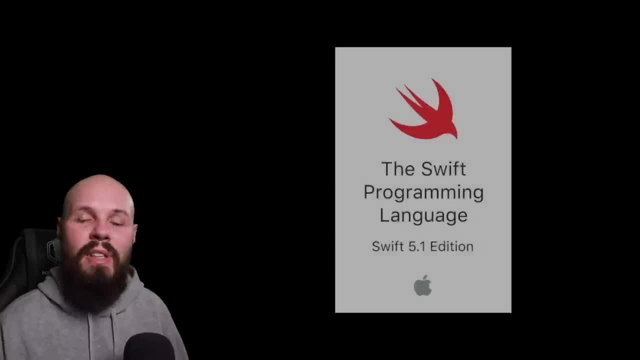 well, But I like Mark's because it's very, very visual. And then, finally, we have the official Swift programming language book from Apple that's free to download. A lot of people will say: start by reading this book. I actually disagree with that because I did that. 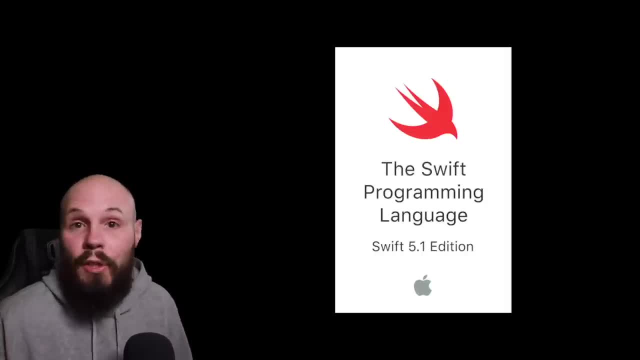 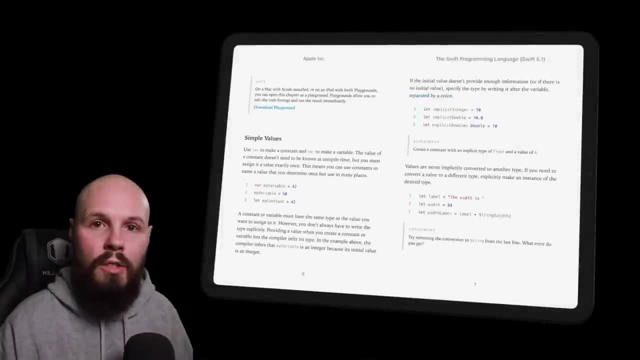 I started and as somebody who started with Swift- like I didn't- I had never coded before. This was all new. That book was just super overwhelming to me because it's very code heavy. You're just, you're just reading a lot of code. 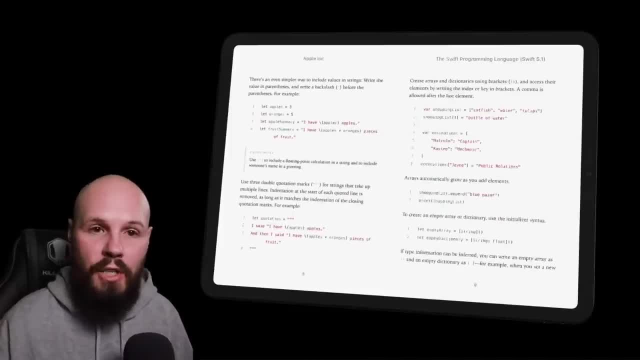 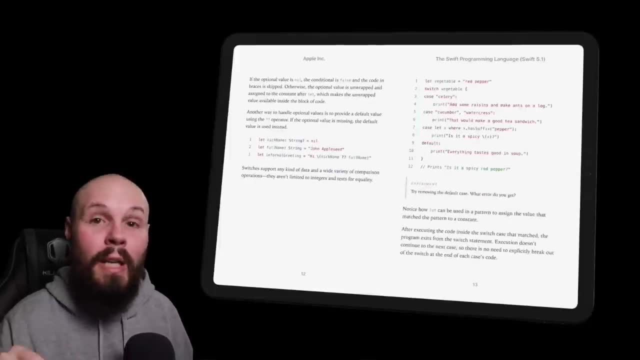 So while I do think this book is great, once you have some like knowledge behind you, I think it can be almost discouraging as like the first thing you read to learn. So I definitely recommend reading this book, but I would come back to it once you've got. 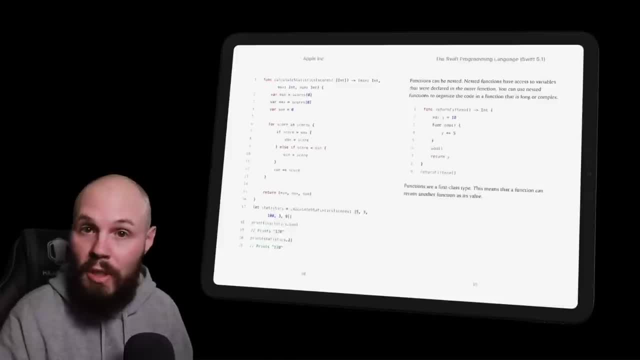 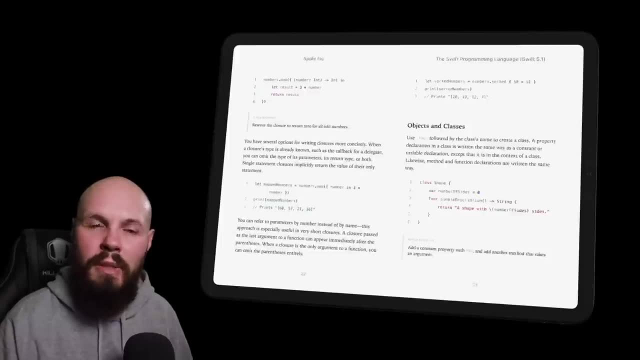 a little bit of baseline knowledge under your belt, And even then, because this book gets into some of the advanced topics. like the advanced topics may still be over your head, But this is also a book that you should probably read every year or two because, again, this 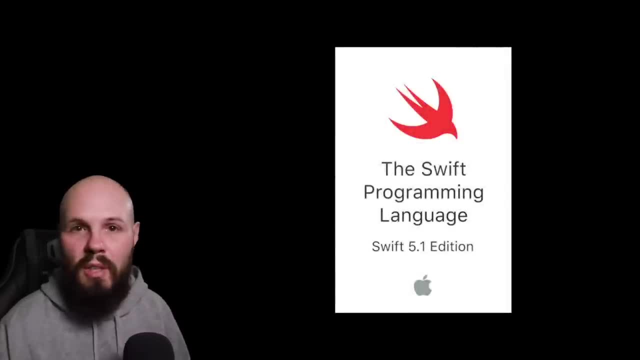 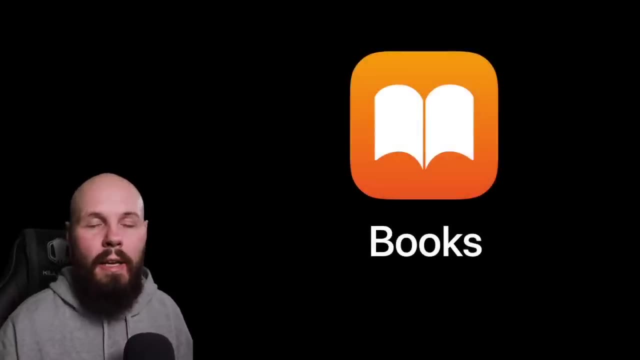 is constantly updated with every new version of Swift, So as new things come out, you know Swift changes. So that's my initial you know kind of group of books, If you're interested in taking this even further. like I said, it was impossible for me to hit. 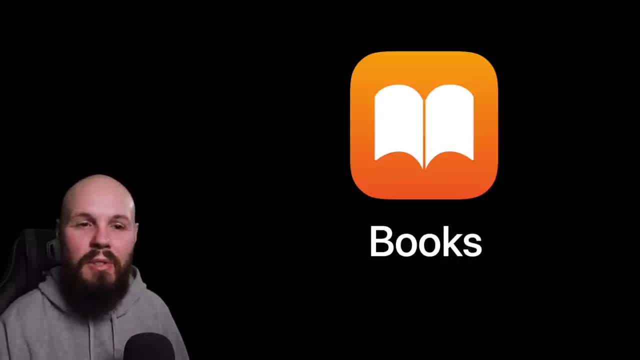 every single book. I know there's going to be some great recommendations in the comments, So please, if I missed one, if you have one, Leave it down in the comments. Leave it down there. And again, if you're watching, don't skip over the comments. 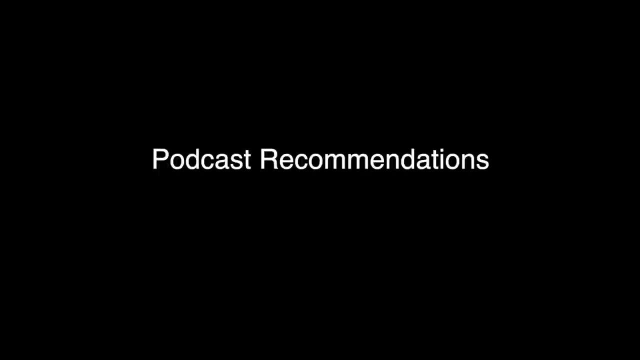 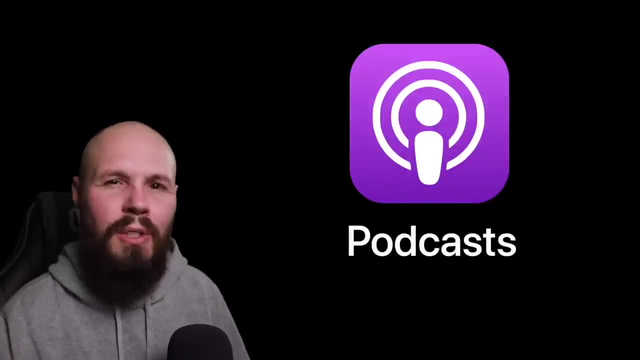 Be sure to check those out. All right, See you in the next video. Now let's talk about iOS developer podcasts. If you're already a podcast fan, you understand how valuable and useful they can be. If you haven't fallen in love with podcasts yet, or you don't really listen to them, I 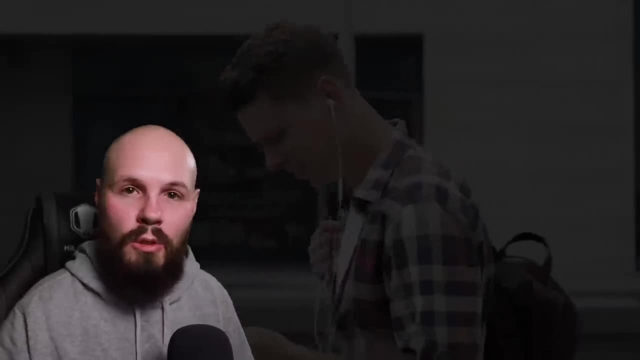 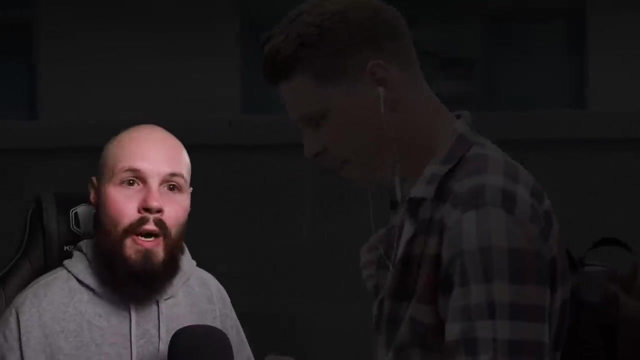 would actually recommend starting, because they're just great on commutes or going for walks. It's great. multitasking because, like you know, you can be learning while you're driving to work. You don't have to be a dog. It's great. 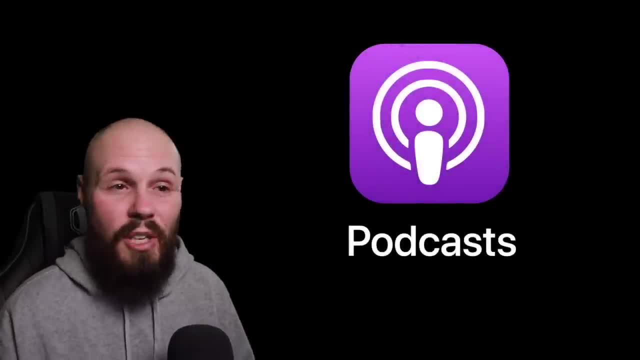 So I'm to the point where I listen to music like 15% of the time. The other 85% of the time I have my AirPods in. it's a podcast. I just love them so much. And part of learning iOS development I believe in like complete immersion. 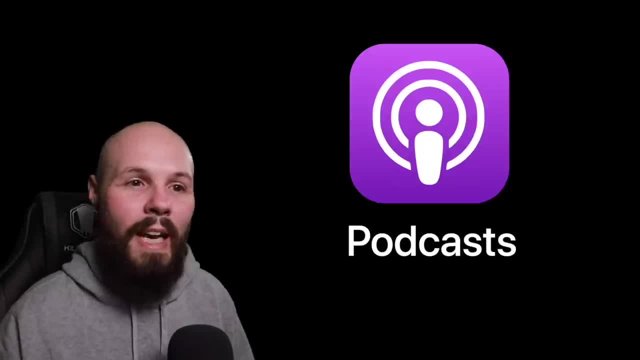 So if you're just learning, you know, always throwing on an iOS developer podcast while you're driving to work or walking the dog, it's just going to help you out a lot. So let's start with some podcasts that you should be listening to. 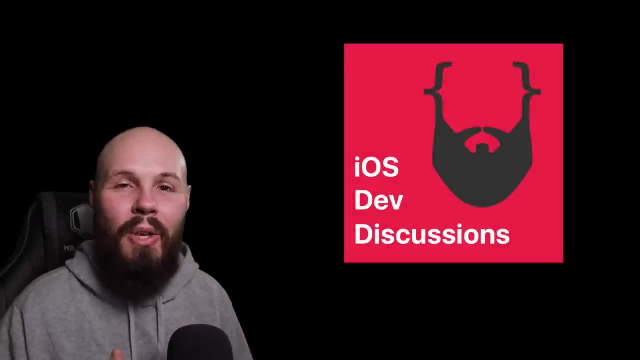 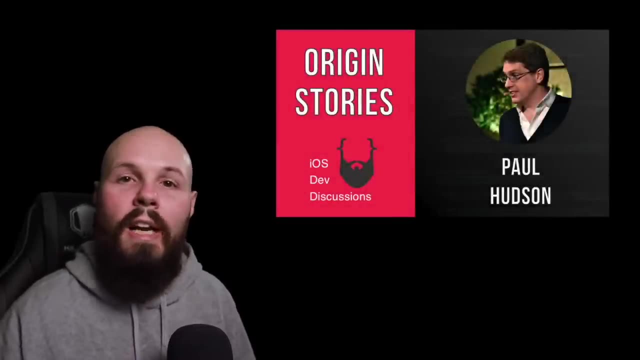 Let's just get this out of the way right away. The shameless plug. My own podcast called iOS Dev Discussions. I do a myriad Of things. I think what most people like is I do a show called origin stories, where I have you know. 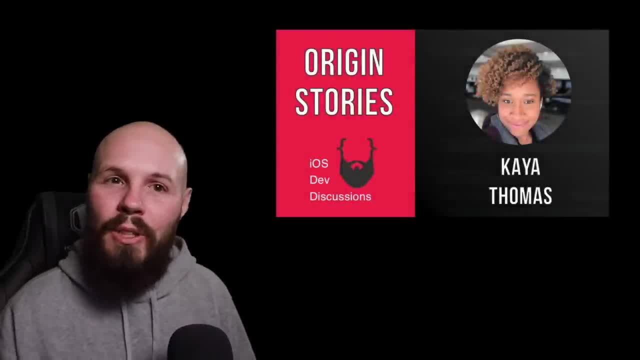 developers. you know, both well-known and not so well-known, on the show And we talk about how they got their start, like right, like what, what? how did they learn to code in the first place? Were they, were they a child? 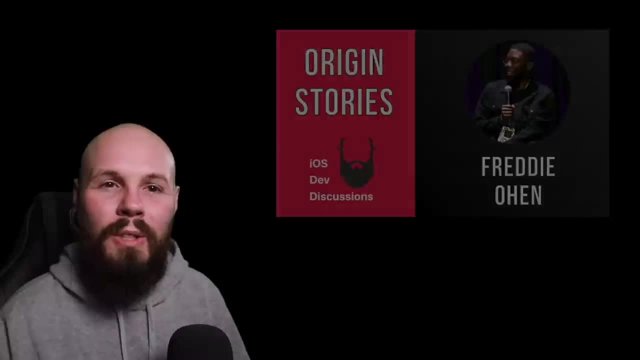 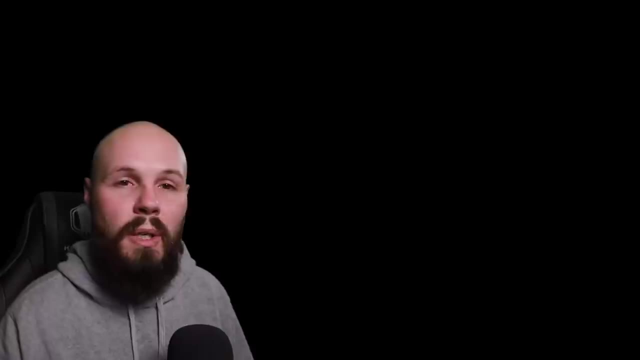 Were they as an adult? Was it via school? What was it that made them want to learn to code? uh, how they went about learning, how they got their very first iOS developer job. again, it's, it's their origin story. 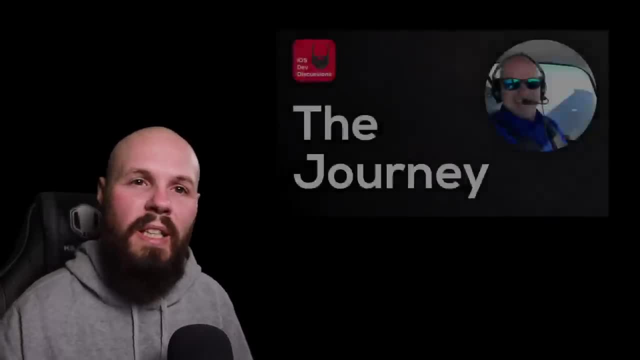 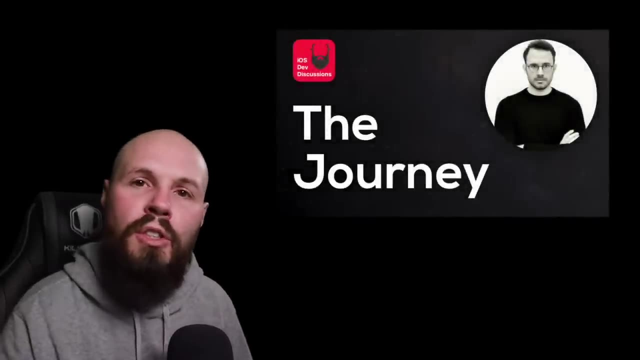 And a lot of people seem to like those- and, branching off of origin stories, I created another show called the journey Right. Bring on people that are just learning And the point of that show is to share other people's journey. you know what they're struggling. 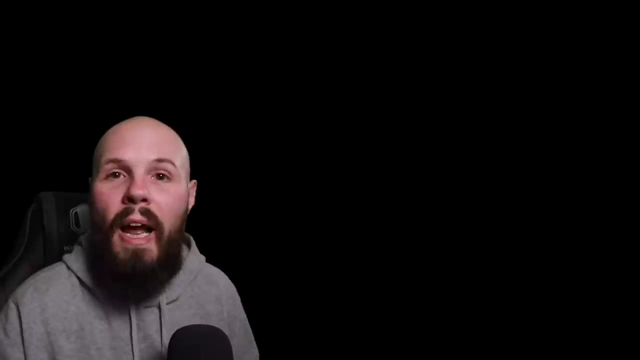 with how they're learning what they're you know what they're doing to to become an iOS developer And, again, hopefully, sharing that story. that information inspires others that are just learning as well. And then, lastly, for my podcast. sometimes I'll pop on for like a quick 10 to 15 minute. 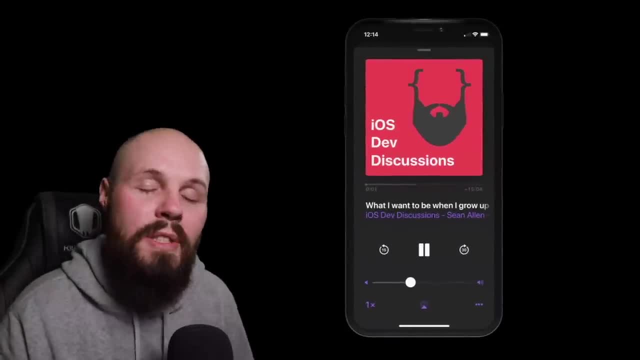 episode, I don't know, just talking about random topics that come to my head, of course, that have to do with iOS development and being a developer. Next up we have Swift by Sundell, which is probably the most listened to podcast in the. 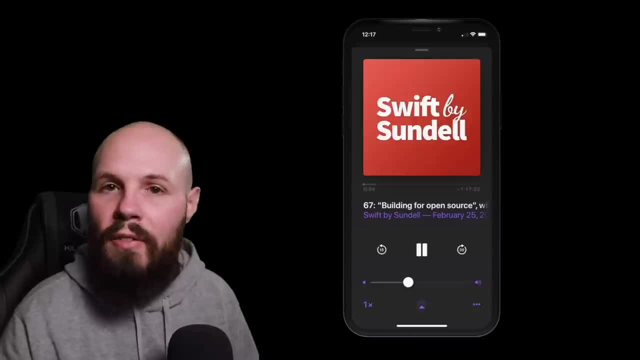 space Like. the numbers aren't public, but I would assume that this comes out every two weeks and he has a different guest on. you know, sometimes it's Apple employees, Sometimes it's other well-known developers. What I like about this show is that he caters the topic of the episode to that guest. 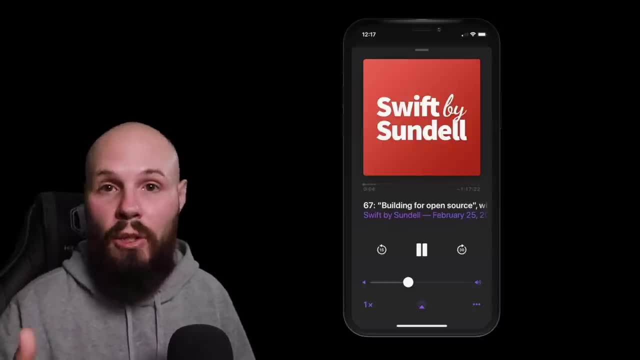 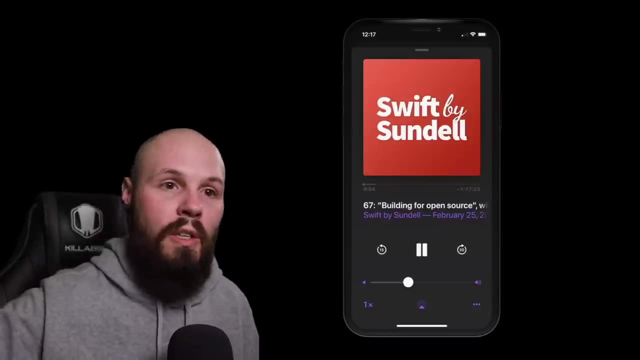 For example, when I was on the show, we talked about content creation. you know, teaching, sharing your, your work, all that stuff, because that's, you know, my strength, That's what I do. However, when he brings on somebody who is very focused in, let's say, machine learning, 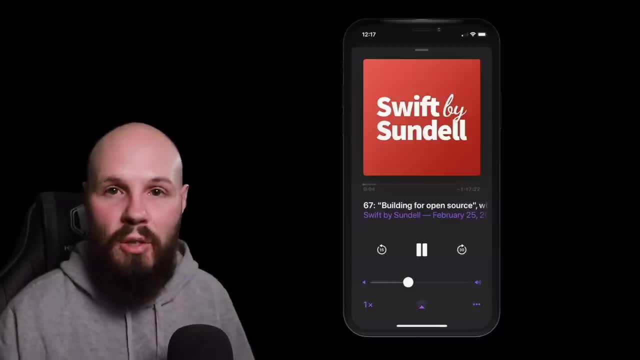 that episode is all about machine learning, So The topics are always different based on who the guest is, And that's why I like it. And it comes out again every two weeks And, like I said, it's probably the most popular podcast in the space. 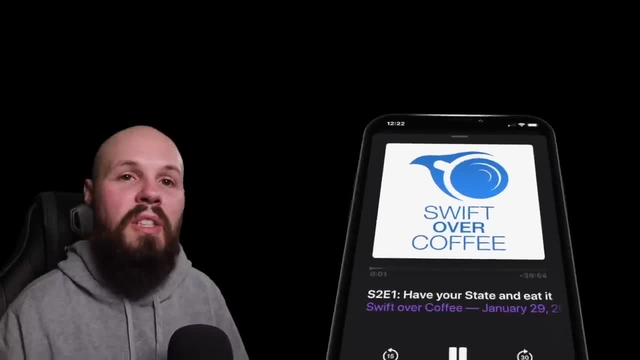 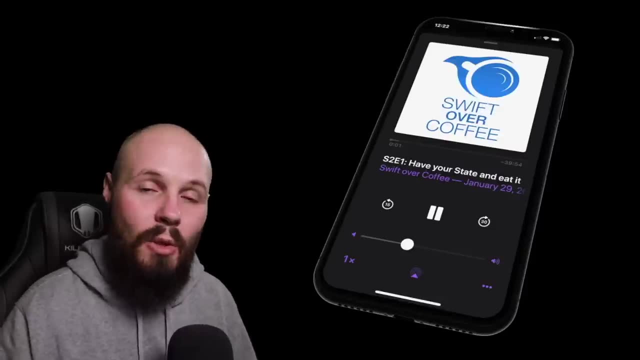 So definitely give it a listen. Next up we have Swift over coffee with Paul Hudson and Erica Sadoon, And I don't think you can find two more knowledgeable people on Swift coming together to create a podcast. So, again, another must listen. 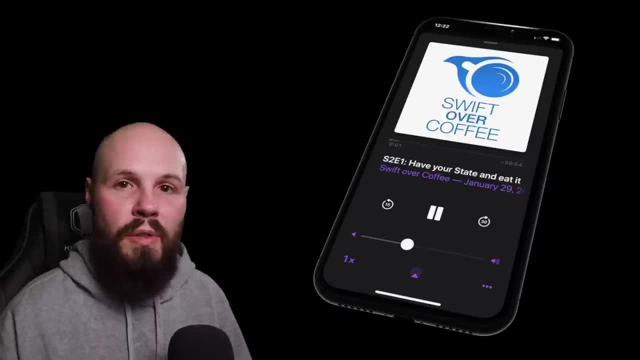 It comes out every two weeks as well, And they break the show down into you know. they do a new section, a pick section, where both Paul and Erica will kind of pick something they want to talk about, And then they do an open ballot section where on Twitter they'll put out open questions. 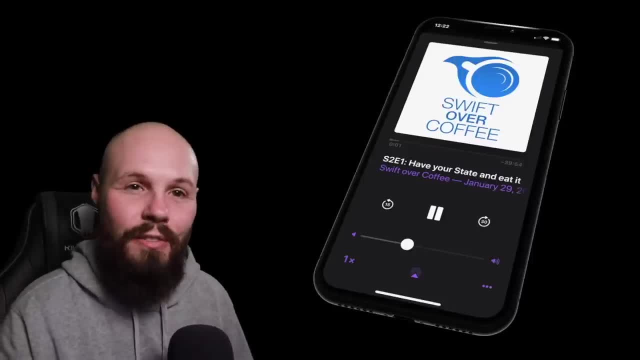 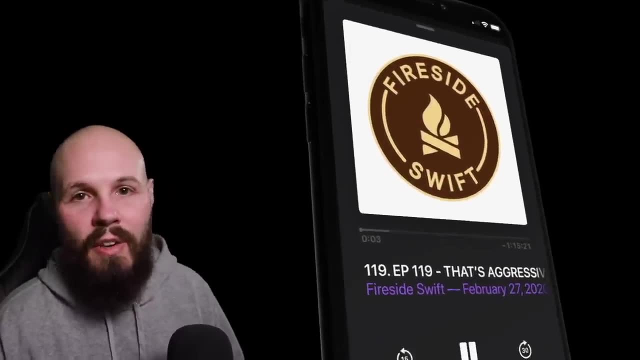 and you can actually interact with the show. It's kind of like the the fan interaction, if you will, asking your Swift questions to again two of the most knowledgeable people in the space. Up next we have Fireside Swift with Steve Berard and Zach Falco. 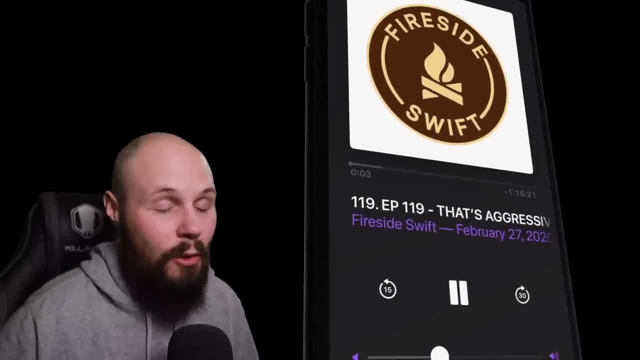 This is a unique podcast because it's very casual and laid back. Don't go wrong. You're still talking about hardcore Swift and iOS developer concepts, But if you just want like a laid back funny conversation where they're cracking jokes having a good time, this is the podcast for you. 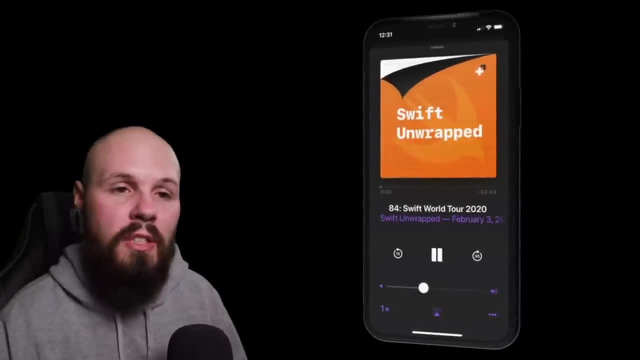 Moving on. This is Unwrapped by JP Smart of Lyft and Jesse Squires. This is a very this is a more advanced podcast, we'll say, because they follow Swift evolution. If you're not familiar, Swift is open source and how they bring in new features into Swift. 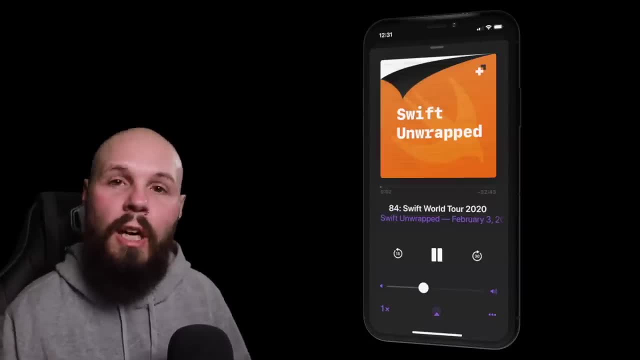 is called the Swift evolution process, where everything happens out in the open and they talk about new features coming into Swift. So this is very like language level development, you know, type podcast and talking about the new upcoming features of Swift. And what I like about it is sometimes they'll even have like the Apple engineers on the 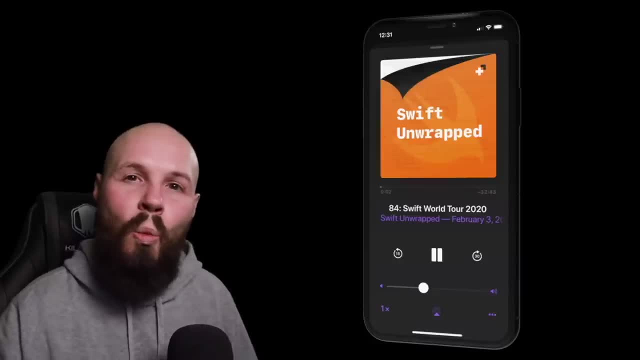 Swift core team, You know, come on the show to explain, you know, why they're implementing these features and kind of the thought process behind all that, which is fascinating stuff. So, again, while this is maybe more of an advanced podcast, you know, for those again this is 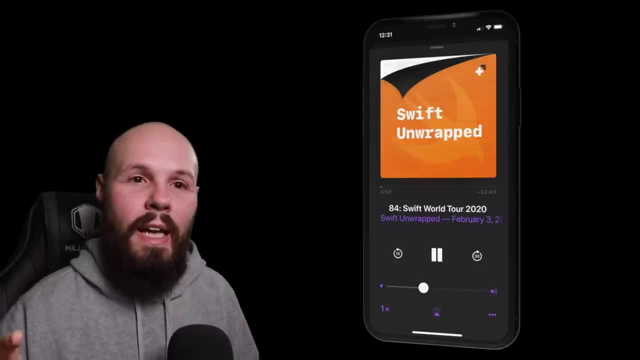 a beginner course, I still recommend putting it on your radar and maybe even listening to it Just again. absorb it, you know, expose yourself to it, But don't be discouraged if, like, 90% of it goes over your head. Even now me, five years into my career, like I would say half of it goes over my head. 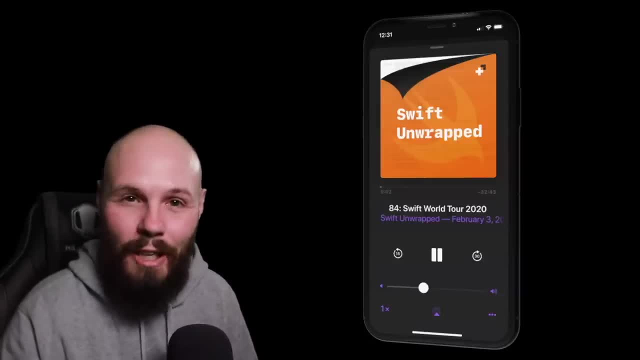 So it is more advanced, but I still think it's great Because, again, what they talk about and who they bring on, and this comes out whenever, like I don't think they're on like a regular schedule, but definitely subscribe to it and 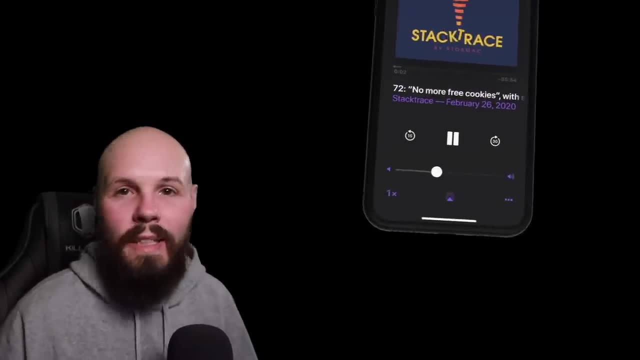 you'll see it pop up in your feed. Next up we have stack trace from John Sandell and Guy Rambeau- again John Sandell's other podcast. but this is life and technology from a developer's perspective. That's their new tagline. 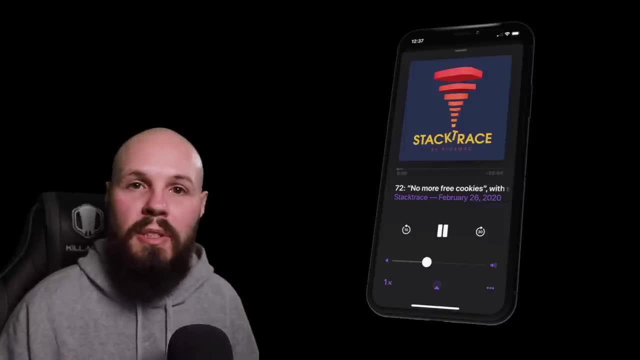 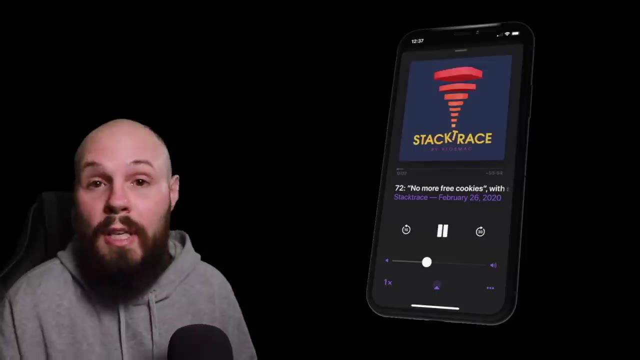 But it's just a great conversation between two very knowledgeable and experienced developers about news like maybe new Apple products coming out and how that's going to affect developers, or like a new framework that's coming out, For example. they're talking a lot about you know like. you know like. you know like. 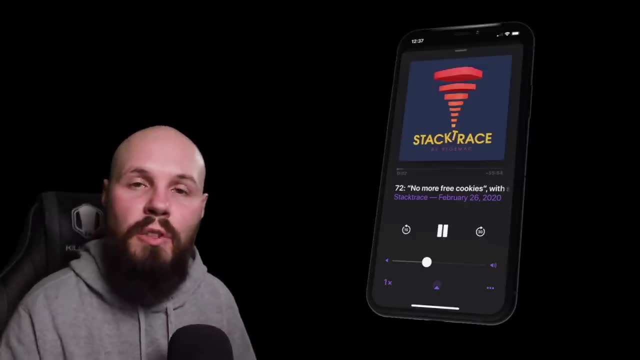 they're talking a lot about SwiftUI lately and their experiences and learning SwiftUI and trying to figure out what is the best architecture because, again, SwiftUI is so new that we're still trying to figure out best practices as a community and they talk about all that kind of stuff. 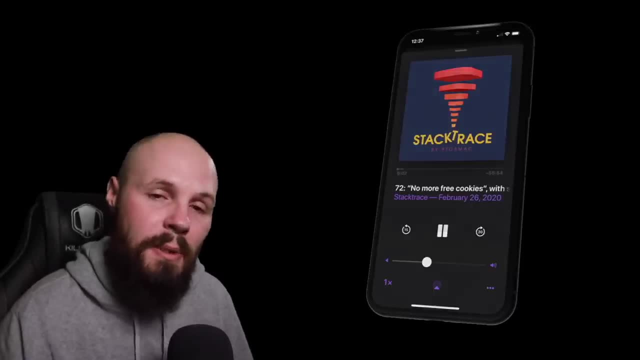 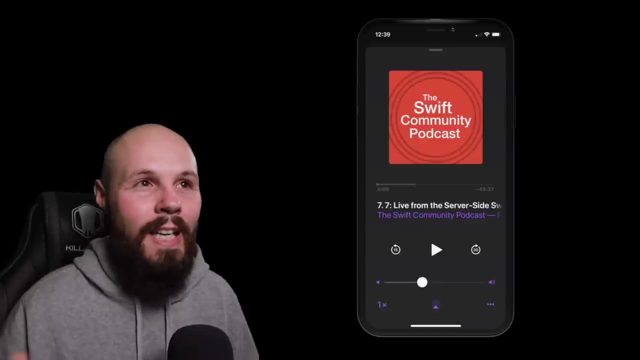 At the end of the day, it's just a good conversation between two knowledgeable and experienced developers. And finally, we have the Swift community podcast, which is a. it's a podcast for the community by the community. It's kind of like a. it's an interesting concept that it's an open sourced podcast, right? 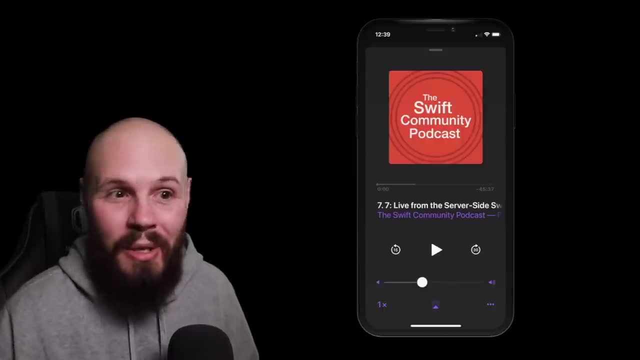 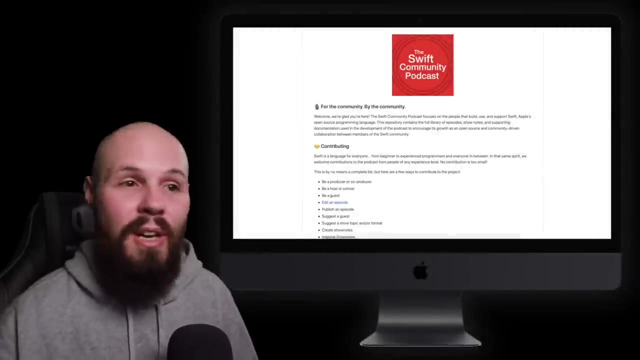 You can submit a topic for an episode. You can even recommend being the host of the episode by submitting a pull request into their GitHub repo. Like everything is done on the GitHub repo talking about lining up guests, what topics are going to do? who's going to edit the show? 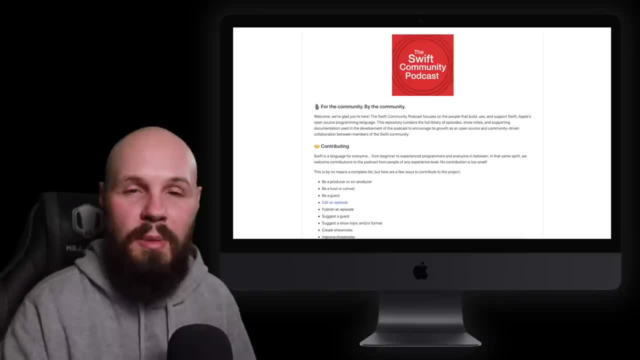 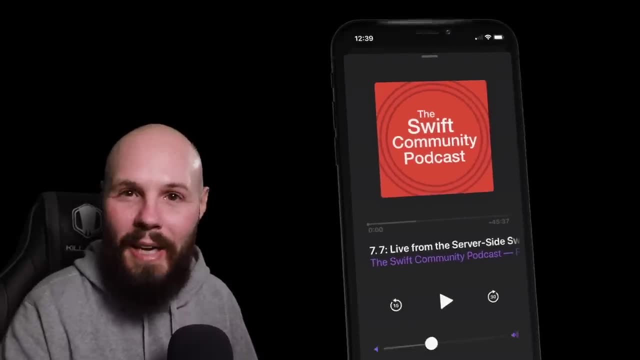 It's all open source, right? It's not just one or two people that run this podcast, So it's a unique concept. Still trying to figure it out. It's still early, It's only been around for a little bit, But it does come out sporadically because, again, it's kind of open source. 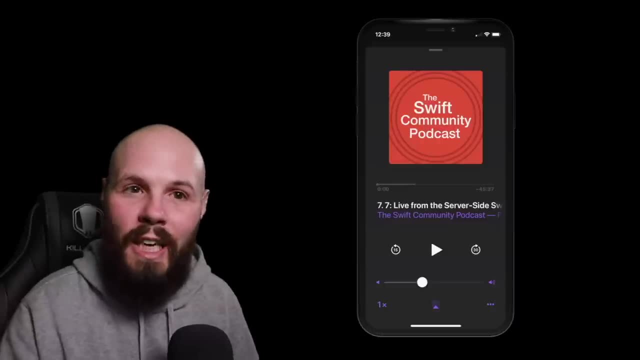 So there's no like set schedule, but definitely check out the repo And if you're interested in kind of breaking into the podcast Space, maybe give it a shot. So those are the main podcasts I listen to. Of course that's not all of them. 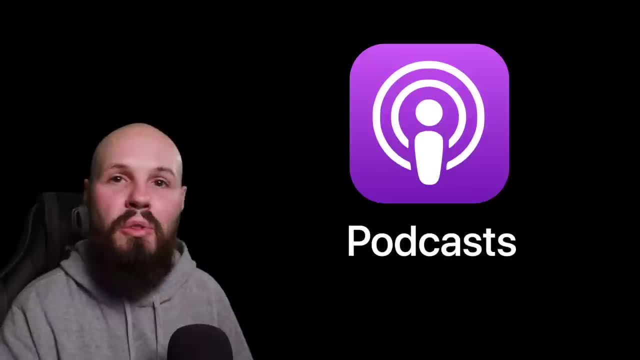 There's way too many to list. So, as usual, if you have a great podcast that you think other students will like, leave it in the comments. And again, if you're watching, don't skip over the comments. I'm sure there's great recommendations down there. 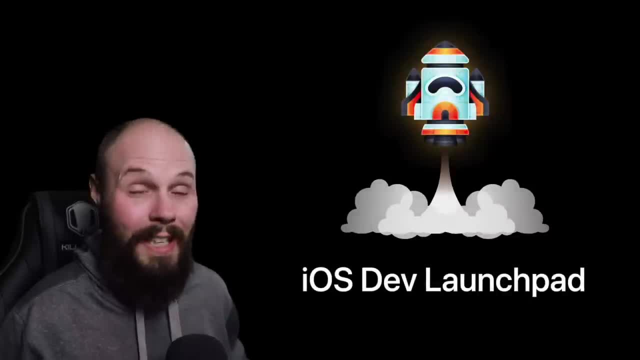 See, in the next video, You just got a lot thrown at you right? I get it Like that was nearly 60 videos of just information. So it is perfectly normal to be feeling a little bit overwhelmed right now and feeling like you don't quite get it. 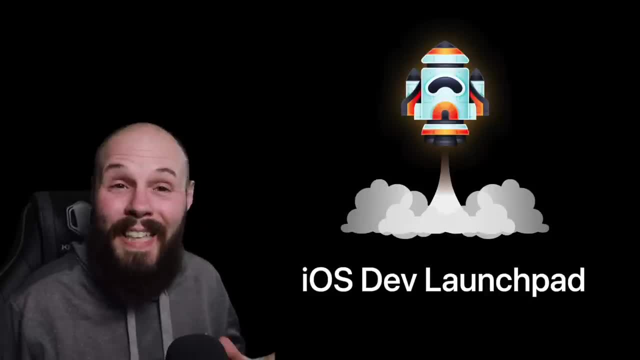 But think about it Like you're learning an entire new skill, an entire new profession, like, and you're just at the beginning, right, You don't watch just a few hours of videos and then now you're good to go, right. 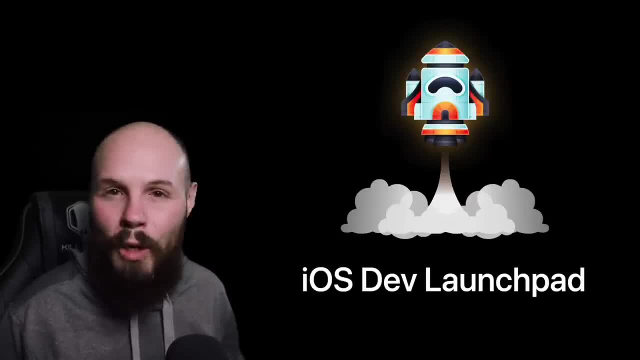 This takes time, Like I keep saying, and like I said, if you feel overwhelmed, perfectly normal. I mean. I remember like when I was doing my bootcamp, I felt insanely overwhelmed. It was like drinking through a fire hose, Like I just was trying to keep my head above water. 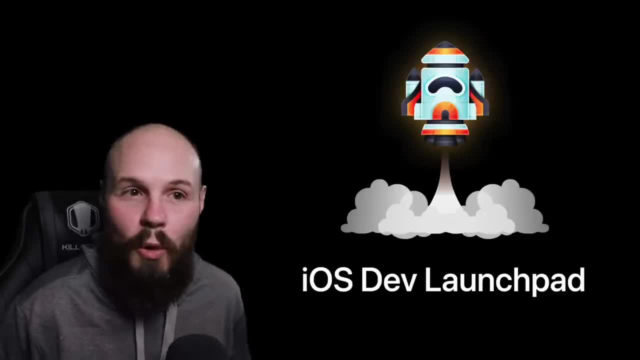 And, to be perfectly honest with you, like I started questioning myself And wondering: like, did I make a mistake trying to do this? Like am I even cut out for this? And I'm so glad that I battled through those feelings Because, again, once you get through that, you're good to go. 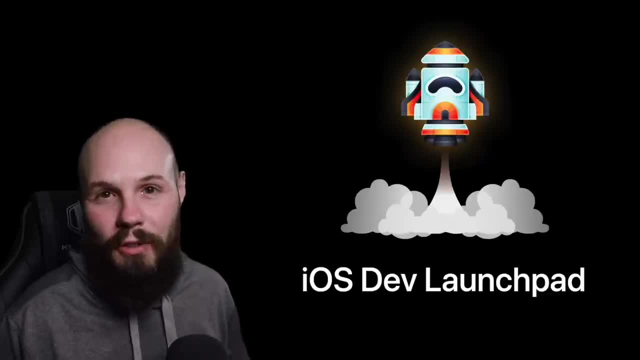 But we've all dealt with these feelings, So don't worry too much. if you're feeling overwhelmed or feeling like, oh man, I'm never going to get this stuff, Yes, you will. It'll just take time. And that's my biggest piece of advice, kind of leaving this course- is to be patient with 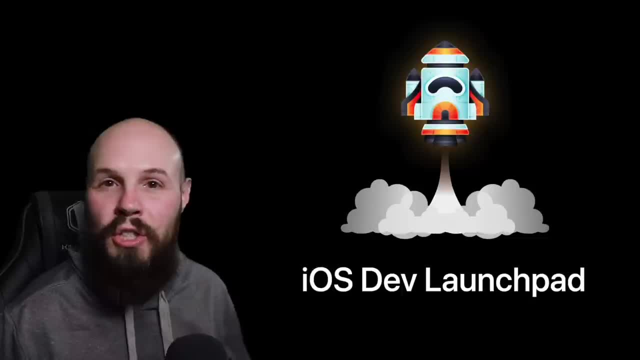 yourself and stick with it. Like I said, this is a very long journey. You may have remembered me saying earlier in the course like six months to two years is what it typically takes people. You're just at the beginning. Be patient with yourself. 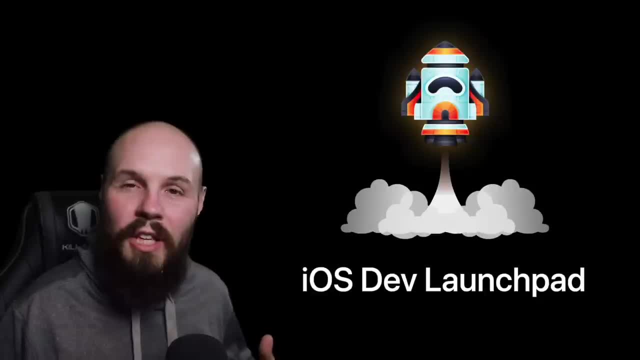 What you're going to see is, slowly over time, like things will start clicking and things will start making sense. And here's the beauty of this course: You own it, right. It's not like you watch the videos once and then you never get to use it again, right? 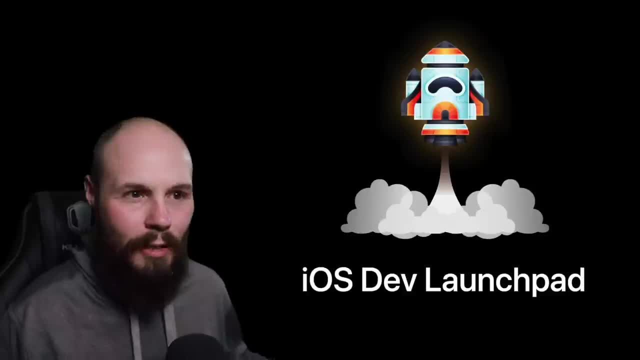 You can always come back to the videos And in fact I recommend it. I recommend going back and rewatching. I like to compare this to Have you ever watched like a really complicated course, A complex movie or a TV show like a Game of Thrones or Westworld, where the first time 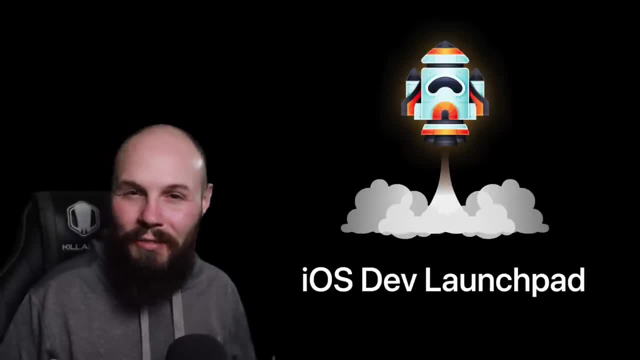 you watch it through, you're kind of like confused and like barely following the plot maybe. But if you go back and rewatch it a second time after you've already seen it, now you start to pick up on the things. Now everything makes more sense and now you understand it a lot more. 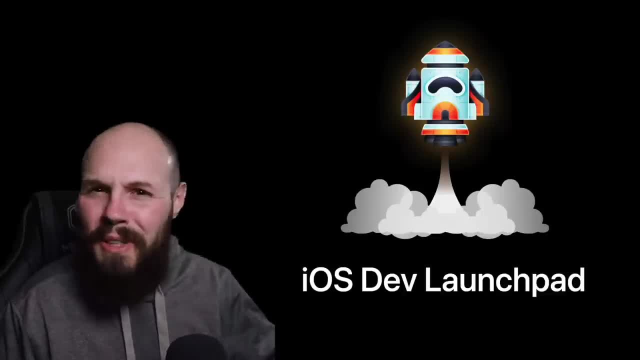 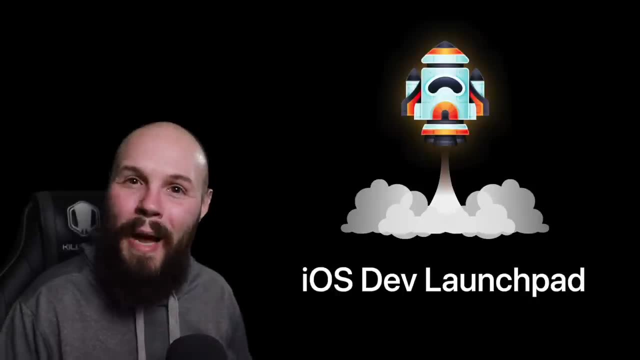 This is the same exact thing. You just watched a kind of confusing and complex movie. So after watching it once, you might be like I'm not really sure where I stand, But if you go back and rewatch it again, you're going to pick up a lot more. 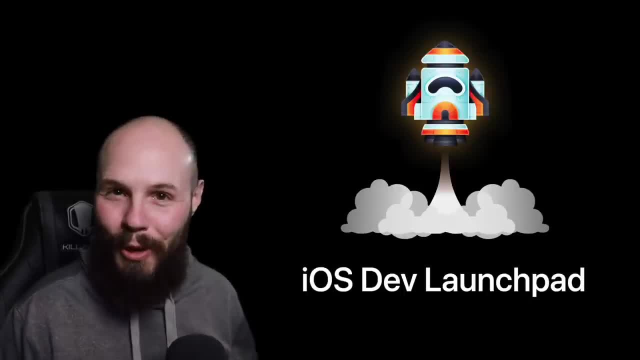 And this overwhelmed feeling you may be having is constant throughout your career. So get used to it. I guess is what I'm trying to say, Because the only constant in technology is change. right, Things are constantly changing And, as a programmer- and you're evolving with technology like you're constantly going to- 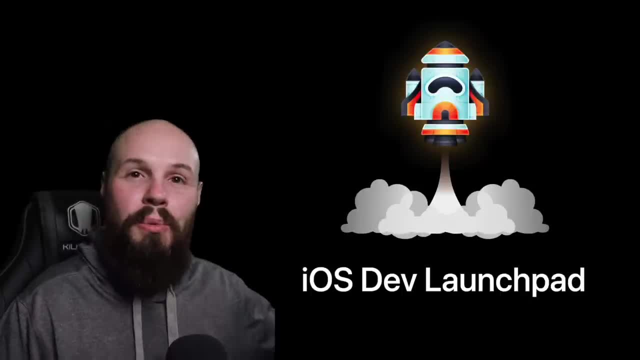 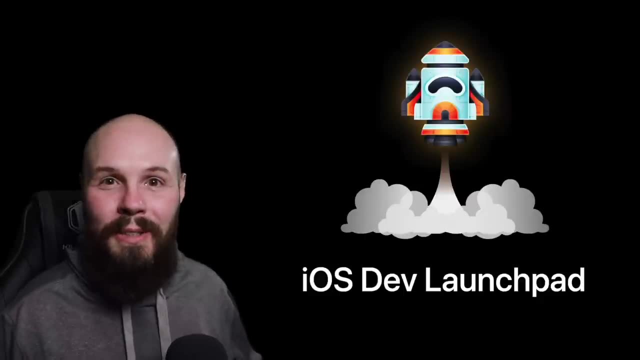 be reset back to a beginner, Like maybe not all the way back to where you knew nothing, But like- here's the example, right Like when Swift was just announced again back in 2014.. Everybody knew nothing. Everybody was a beginner in Swift. 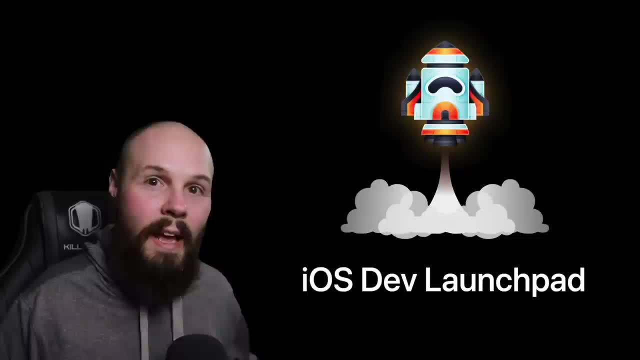 Even just recently- summer of 2019,, Swift UI was announced. Everyone was a beginner at Swift UI, So what I'm trying to say is: get good at being a beginner, because that's going to be constant throughout your career, and kind of learn to deal with and evolve with this overwhelmed. 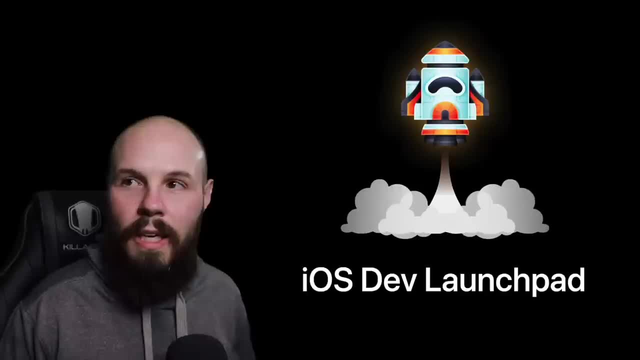 feeling Because you always get it. every time you learn something new And I think the key there is having the determination to battle through this overwhelmed feeling, Like I know some people like aren't willing to go back and rewatch videos Or do a tutorial twice right. 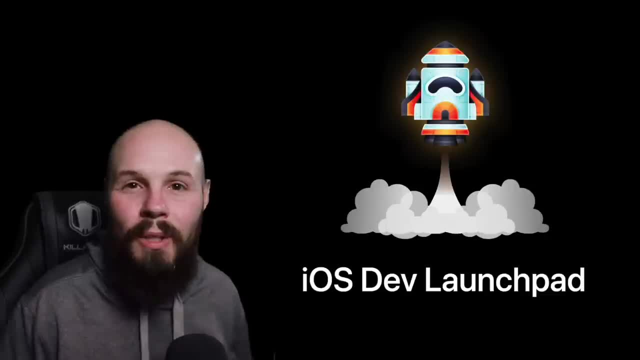 They think they can just watch it once and then they know it Like. that's just not how it works. It's like any other skill: You have to practice and drill the fundamentals. So at the end of the day, don't worry about being overwhelmed. 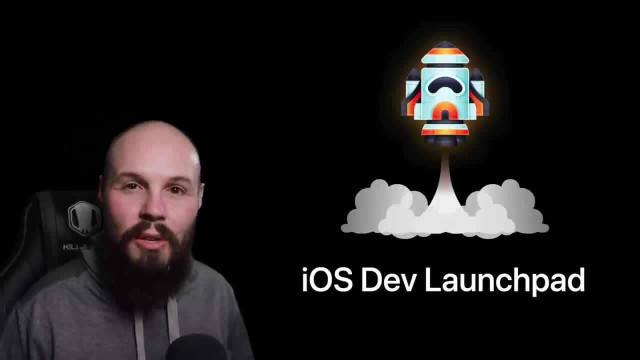 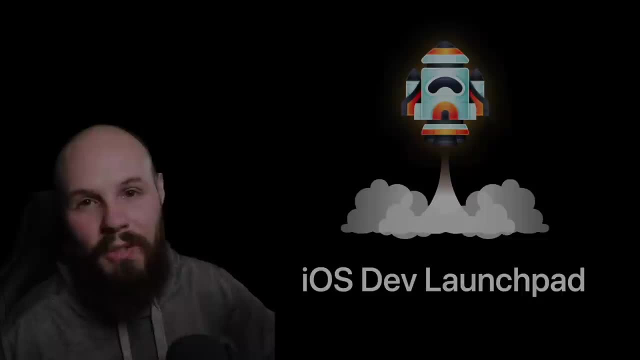 We've all felt this. It is perfectly normal. Be patient with yourself, Keep going, Take it little by little And I guarantee you six months later you're going to look back and you're going to be amazed at how far you've come. 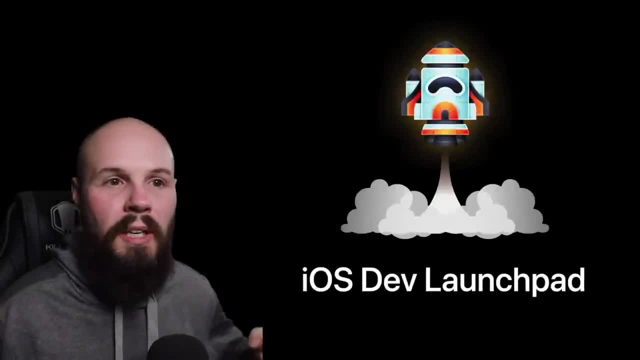 So here you are, wrapping up your beginner course, And you're probably wondering: all right, what's the next step? What do I do next? And well, my first answer you might not like, but what I'm going to recommend if this was. 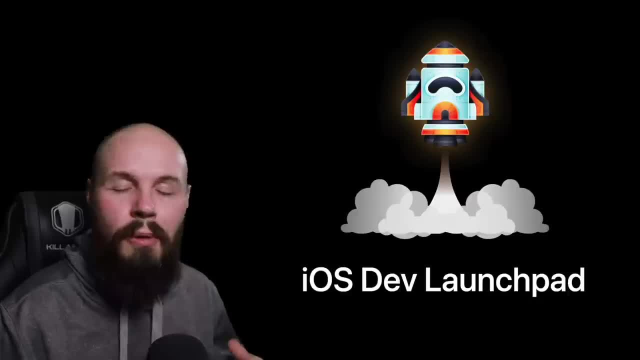 your very first course. you know, if you have a little bit more experience- and this was reviewed for you, maybe not, but if you were the absolute beginner and this was like one of your very first courses, I'm going to say run it back. 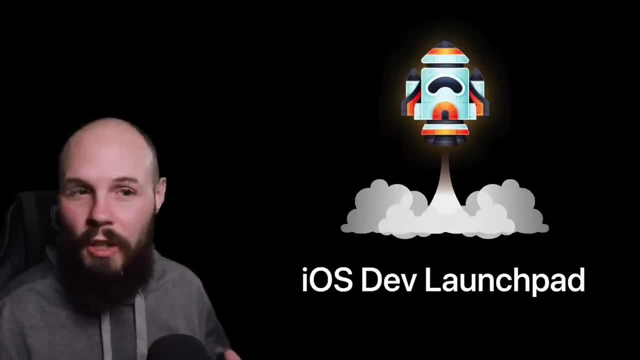 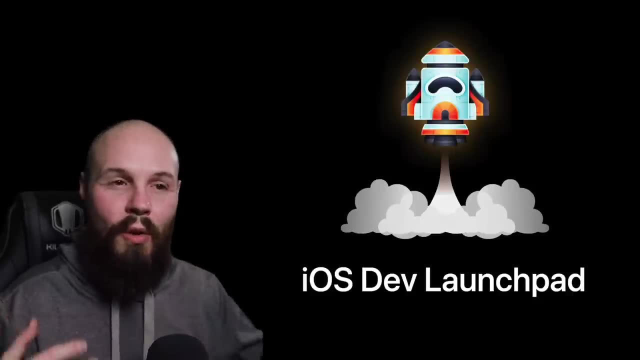 Like I mentioned in a previous video, you just watched a pretty complex movie. Go watch it again And you're going to learn a lot more. You may not have to type everything out, but at least rewatching the videos once you have. 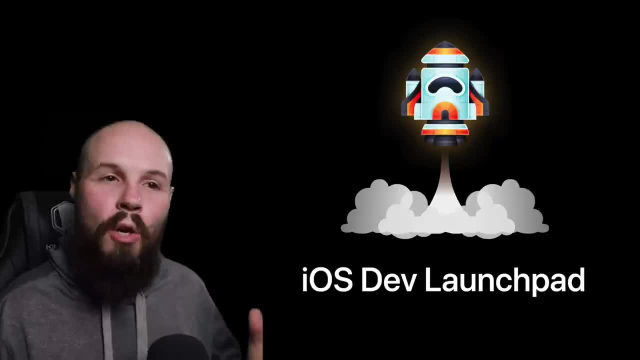 all this knowledge, It's going to help you out a lot more. And I say to go run it back and rewatch those because I want to instill the habit, or maybe the lack of stigma, that going back and rewatching videos is not a bad thing. 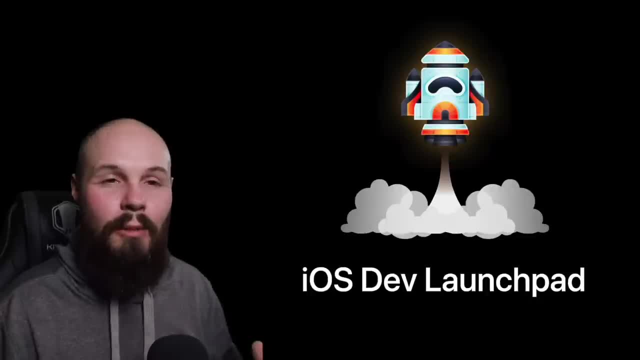 Like doing a tutorial twice, not a bad thing. Like I keep saying, repetition is key. You have to drill the fundamentals, Like this is how you get good at things. Think of something you're good at, I don't care- Video games, sports writing, whatever you are good at, 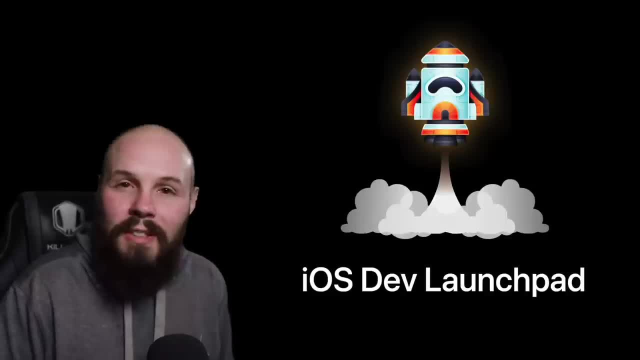 Did you just do it a couple of times and then you were good at it? No, You missed it for months, years, whatever, and then you got good at it. This is no different. So what I'm going to do is go back through the videos and add links to blog posts or 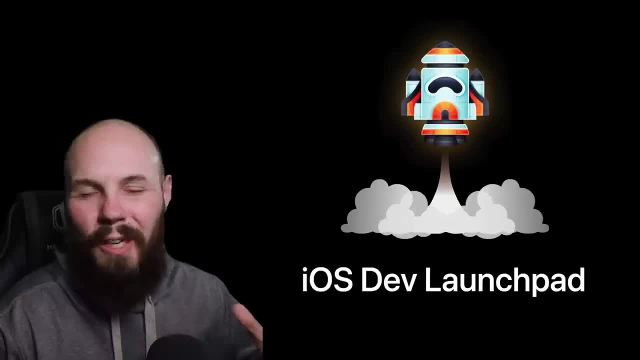 other learning resources on each of the topics, if it's applicable. Not all videos may have these links, but this is a way for you to go back and learn more about that specific topic, And this will be other people's blog posts, et cetera. 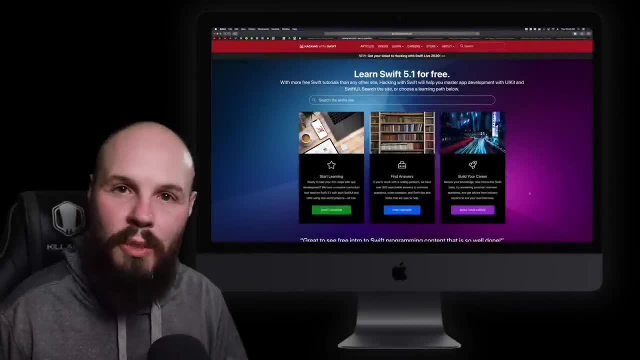 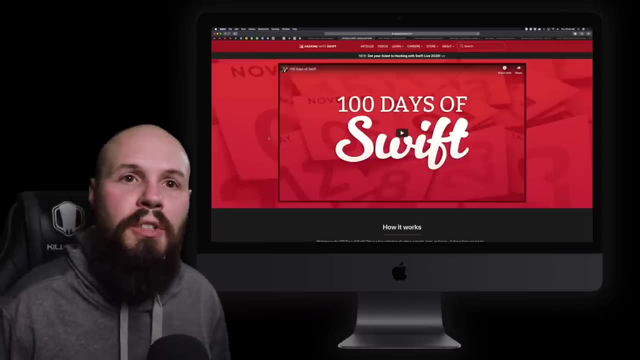 After you've revisited this course, I would recommend going to either hackingwithswiftcom or raywunderlichcom. We talked about this in our iOS resources section of the course, So hopefully those names are familiar to you, But they both have beginner content, whether it's books or videos. 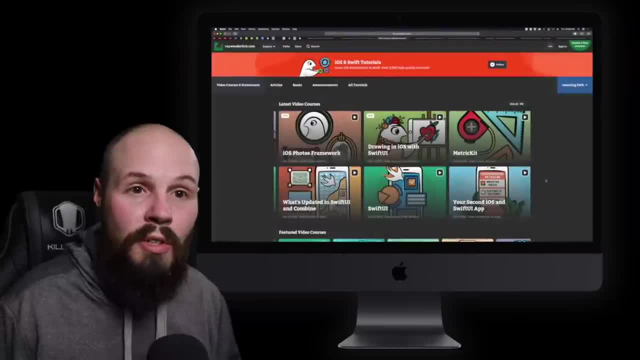 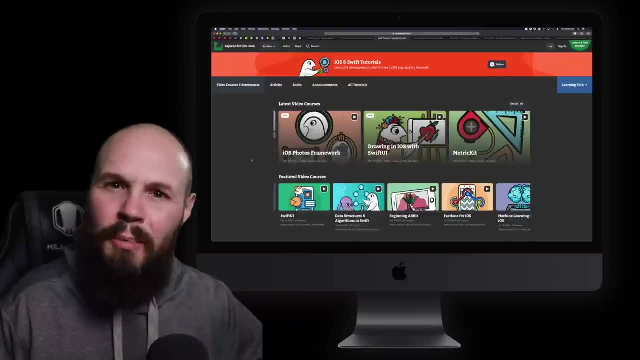 I recommend going through that And even though there will be some crossover, some of it will be repetitive. what I have found when learning is that oftentimes hearing a different teacher explain something a different way will make things click, Because not only are they explaining it a different way, but you're coming into their 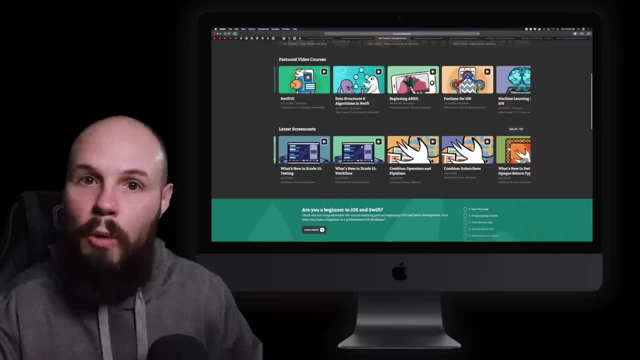 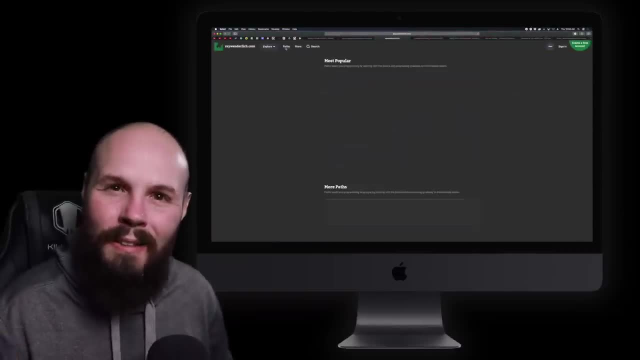 content with some preexisting knowledge from this course, Or maybe, if you've done their stuff first and you came to this one, Just hearing things explained different ways Can really be helpful to make that click. And then after that, I may or may not have released this, but I have plans for what I'm. 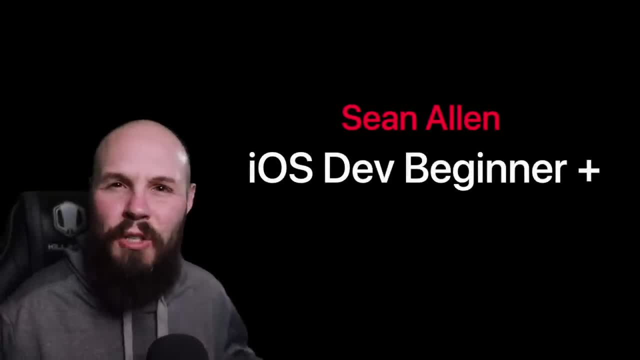 calling a beginner plus course, And that is the next logical step on concepts after this course. If you're watching this in the first half of 2020, it's not released yet. I plan on releasing this in the second half of 2020.. 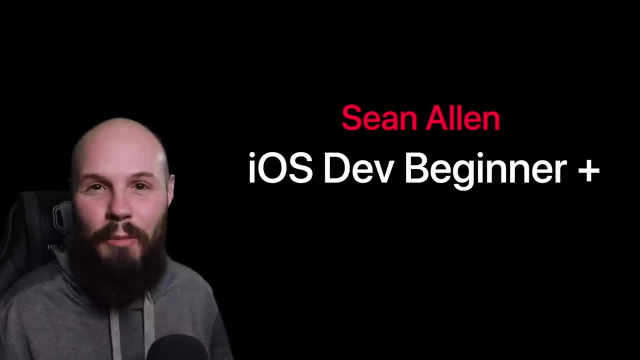 So, depending on when you're watching this, if that's available. But if that is available, again, I'm designing that course to be the immediate next step to this course. So that might be a great next step, If not, again check out Hacking with Swift or Ray Wunderlich. 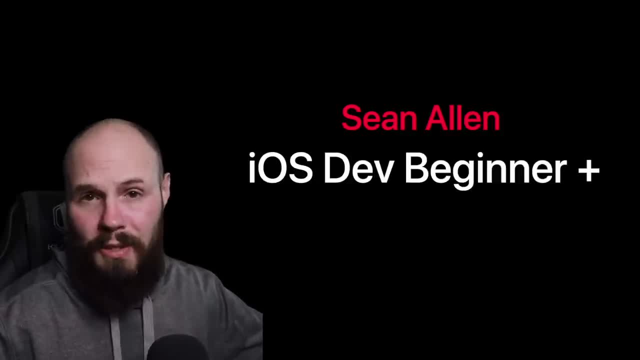 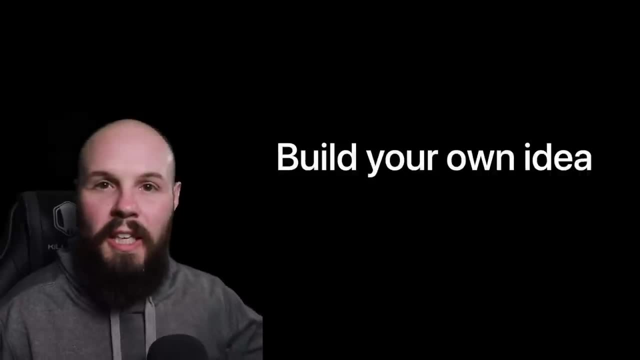 Again, check them out regardless. They have great stuff. Actually, you may have heard me say Ray Wunderlich back in 2015 is how I got my start, is how I learned. Now, after you've explored some of these beginner content, again, Hacking with Swift, Ray Wunderlich. 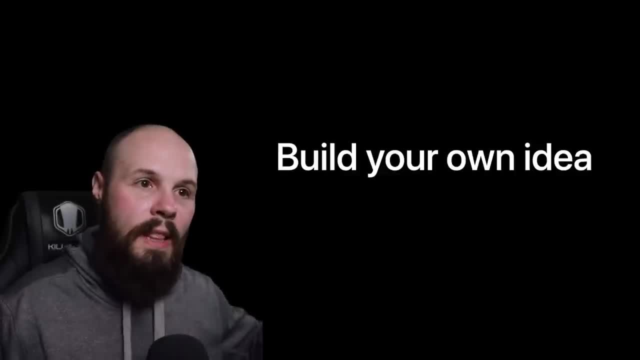 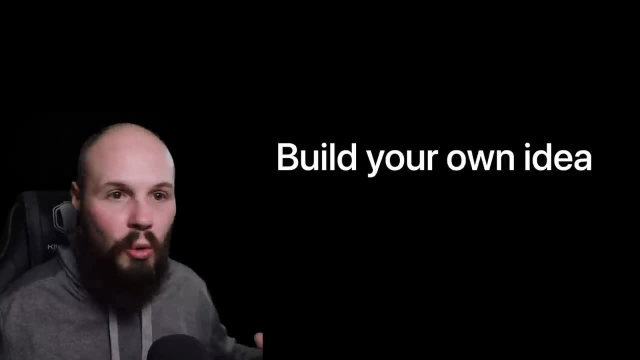 my stuff and some of the other resources I've put out there. the next big leap you're going to take in your learning is to create your own project. Now I want to be clear. This does not have to be a world changing app. 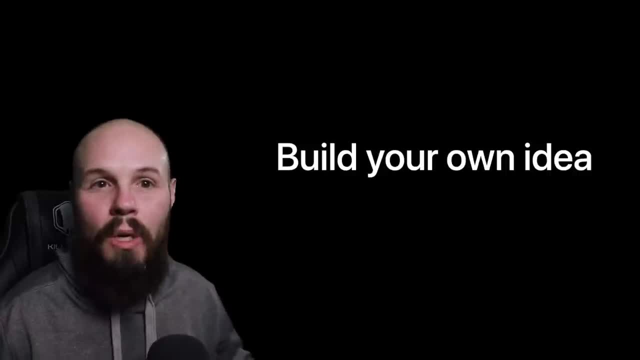 You don't have to create the next Instagram. This can be dead simple, But it needs to be your own idea, Something that you're not just following a tutorial on, Something that you say: I have this idea, How can I bring that idea to life? 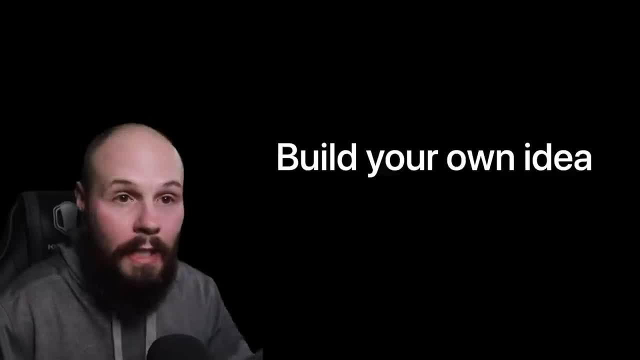 And you have to do the research in between to make that happen. But again, it can be super simple And I actually recommend that it's simple. If you do think you're going to build the next Instagram and you concoct this crazy complex app, you're biting off more than you can chew. 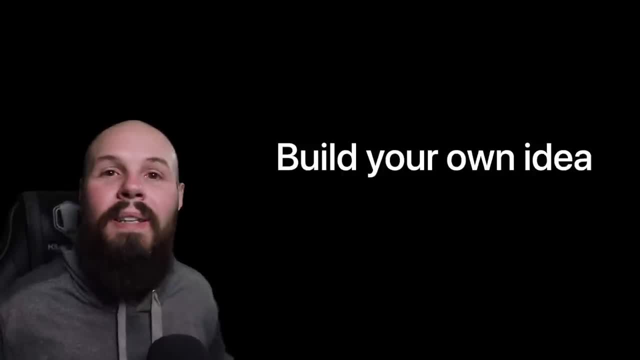 And that is very likely, you know. of course you could pull it off, but it is very likely that that is going to be more discouraged. Then helpful again: baby steps, long journey, little by little you'll get there, but building. 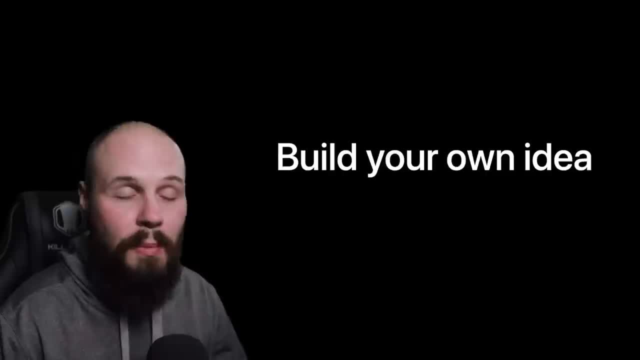 your own project And again solving your own problems where you don't have a tutorial that spells everything out for you, your learning will accelerate immensely And that is you taking the next step in your journey. Then, once you have the solid foundation, you've done those beginner courses, you've kind of 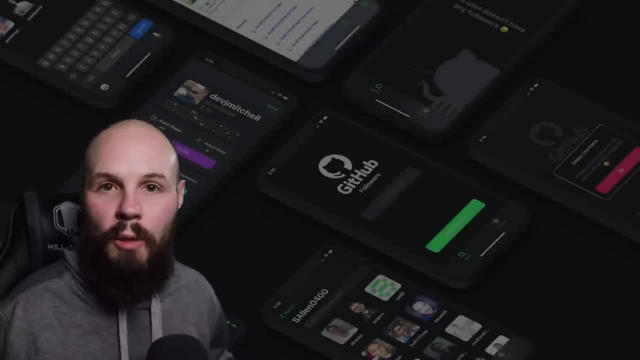 built your own project. I would recommend coming back to my iOS developer take home project course, the GitHub followers course, Because that course was designed To be like The final boss before you start applying for your first real iOS developer job. That course is based on well a lot of times. when you're interviewing, the company will 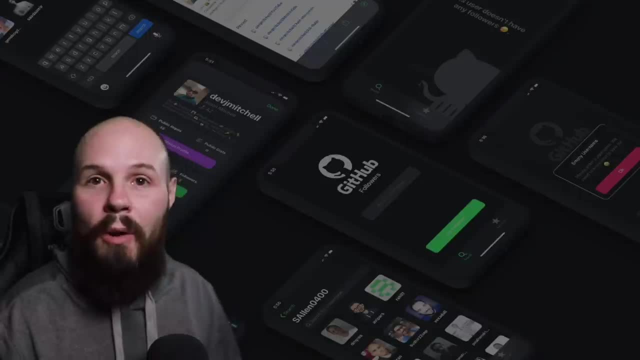 send you a take home project and they'll say, Hey, you have whatever three to five hours, build this project and send it back. And we kind of mimic that whole process, except we go a lot more in depth Because, again, this course is preparing you for the job interviews. 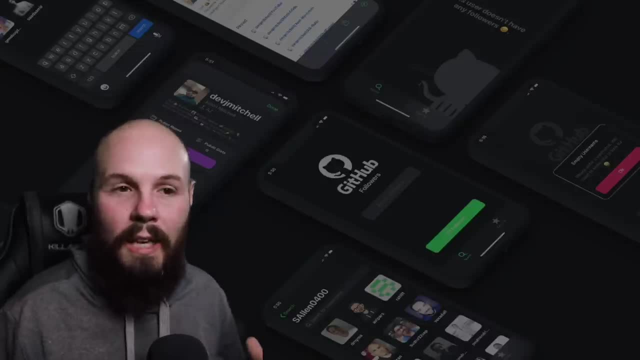 So we cover a lot of the main topics that are typically asked in iOS developer job interviews. So, like I said, doing that course Was designed to be like the final boss before you start applying. it's meant to prepare you for those junior developer job interviews. 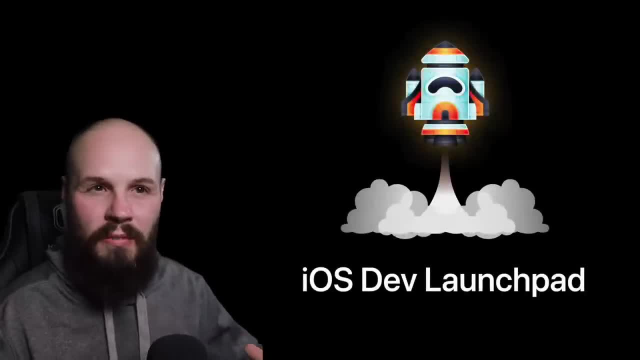 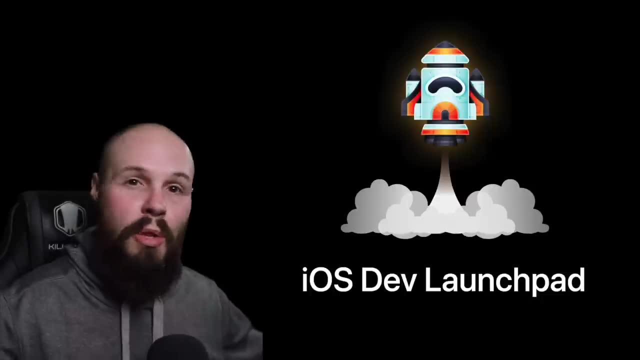 Now, of course, everyone's path is going to be different. The path I just laid out is very vague and rough. right? You did this beginner course. If my beginner plus courses out, take that Even if it is out. explore hacking with Ray Wunderlich and some of the other iOS developer. 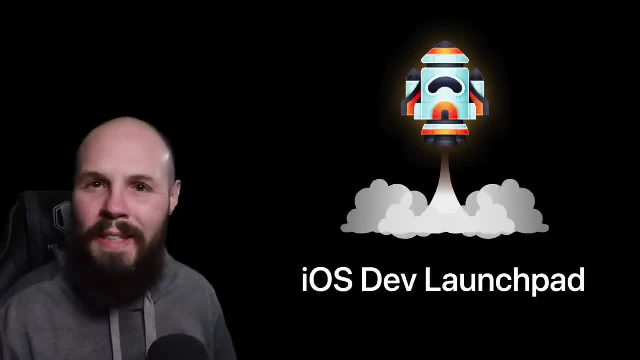 resources I put out there. Then start building your own project, your own idea, Keep the app simple, Then kind of round it back to my iOS developer take home project. That's the rough vague path. That's the rough vague path, But again it's vague. 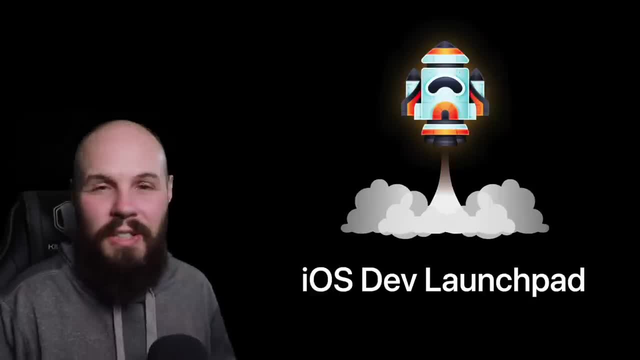 Make it your own. You don't have to do exactly that, but that is a good roadmap, if you will, to potentially have your full-time job, be an iOS developer And, along the way, again, be sure to partake in the community. 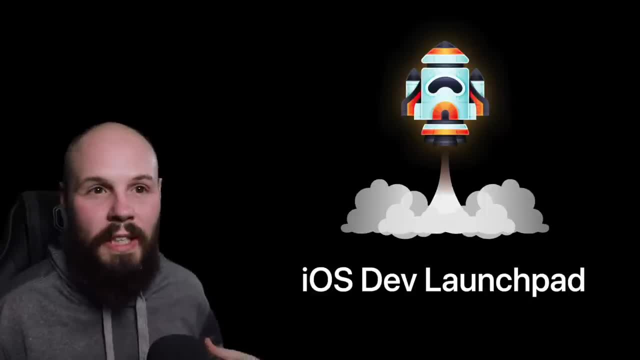 That's one of my biggest regrets. I didn't start partaking in Twitter and interacting with other iOS developers until I was like two years into my career And I look back, that is one of my biggest regrets. So I implore you, don't be afraid, hop in the Slack channel, start interacting with. 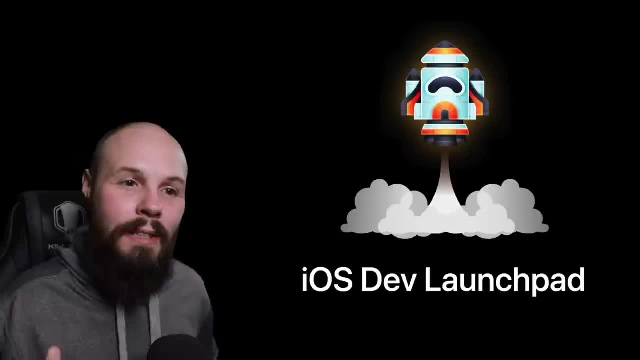 us in there Again. interact on Twitter, Like I say in my Twitter video. Trust me, that will pay off in the long run. And then, finally, like I said before- I want to stress this- Just be patient with yourself. 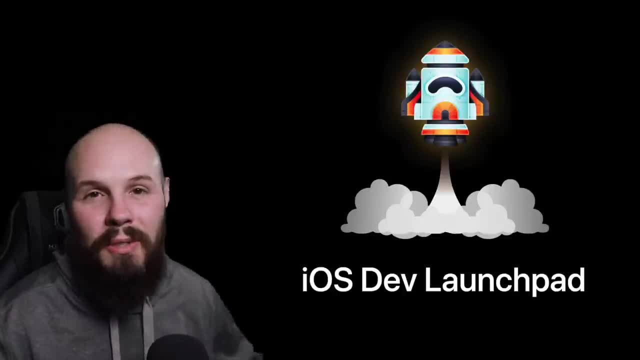 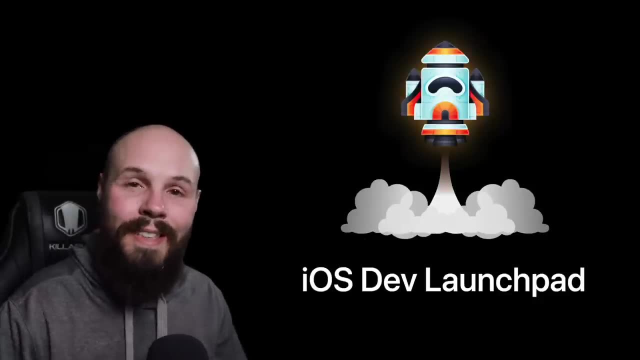 Again, this is a long journey. You've heard me say six months to two years typically, And I've seen it firsthand. People that have been following me and my YouTube channel. I've watched their whole journey go: from I'm just learning to now they're hired full-time iOS developers. 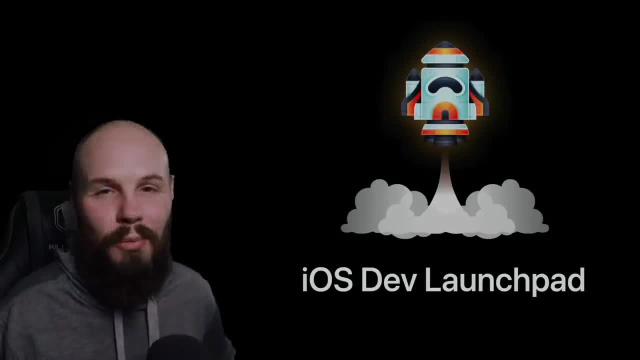 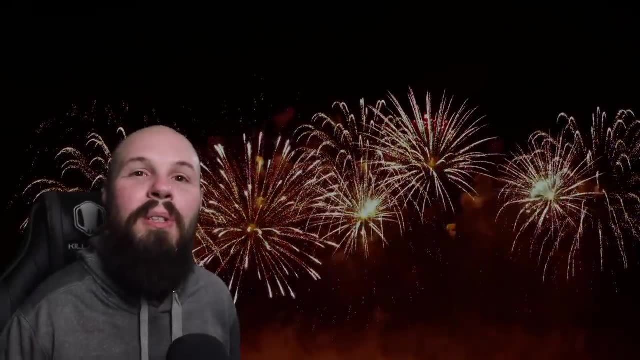 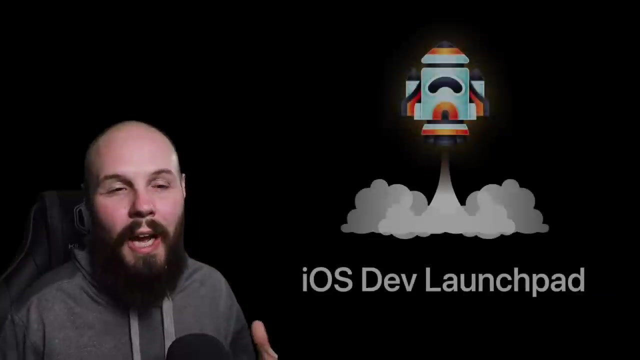 It happens every day. So again, be patient, it's worth it. Congratulations: You've completed the course, You've officially begun your journey, Your rocket's taken off. It's exciting times, And I do want to take a second to sincerely thank you. 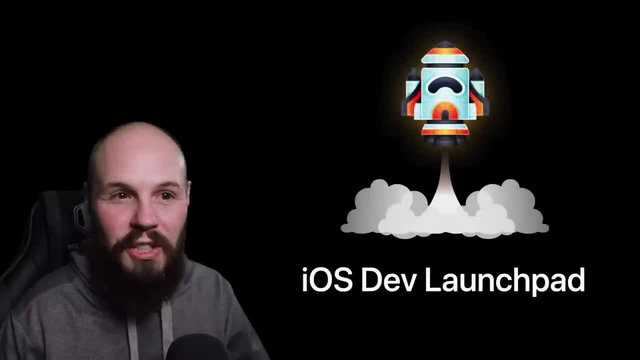 I really enjoy teaching this stuff. I love watching the progression of the students, be it via the comments or the Slack channel Watching students have that. I call it that click moment where you can see the light bulb go off and they finally get it. 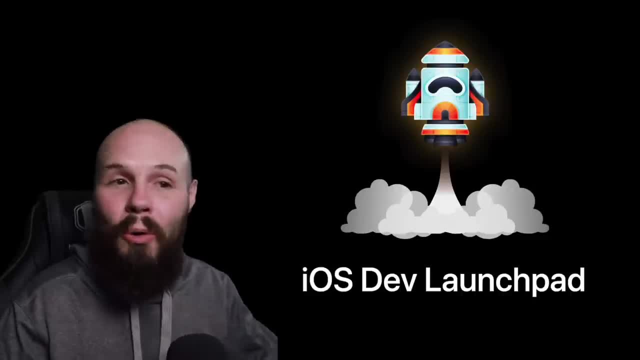 That's the value I get, So I hope you got value from this course and you may be thankful to me for teaching you. Just know that I'm getting just as much, if not more, value from this course, And I'll see you in the next one. 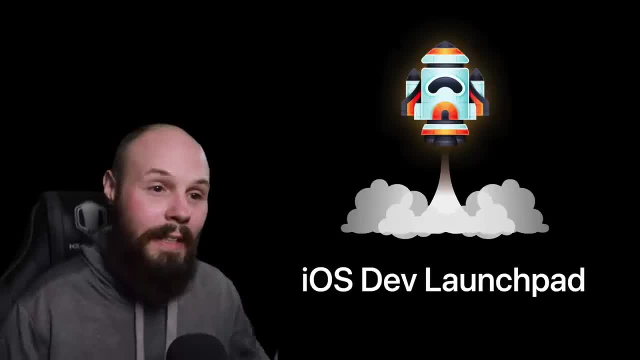 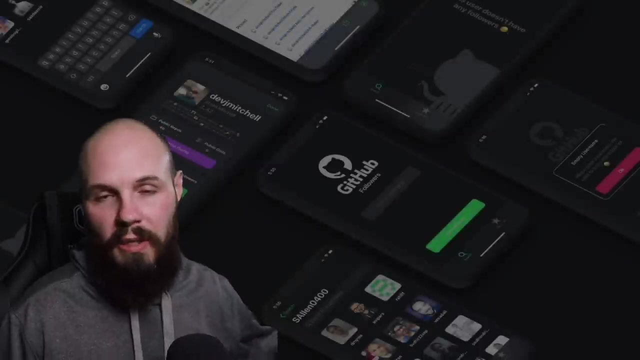 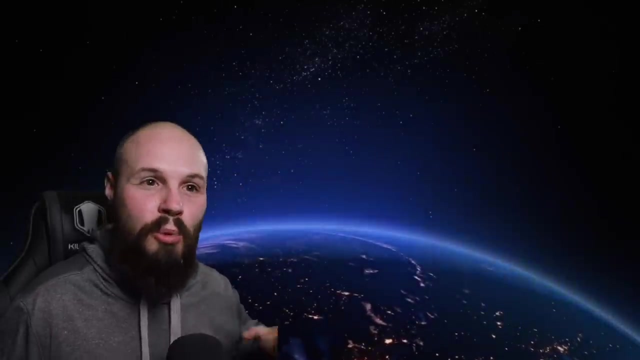 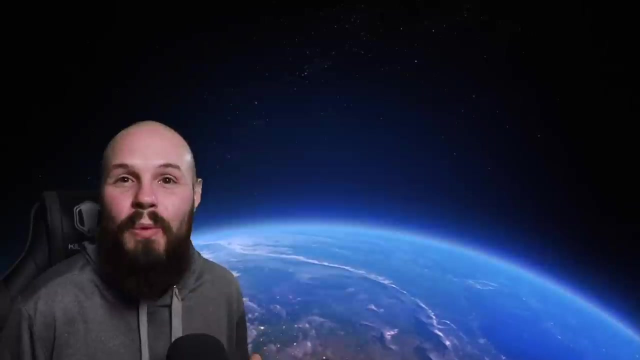 Bye for now. Bye the best, most premium iOS developer courses. frankly, in the world. I know that's a lofty, audacious goal, but that's what I'm striving for. So I'm absolutely not there yet. Again, this was just my second course. 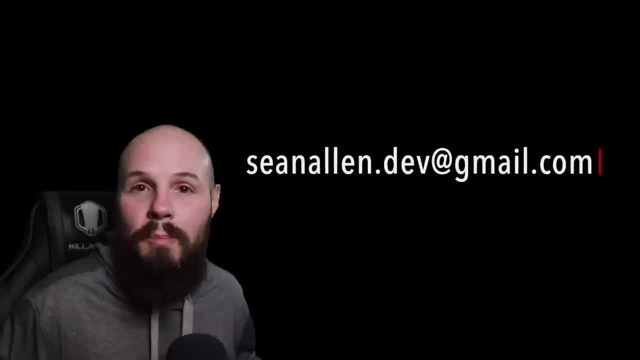 but what I'm gonna ask of you- and here's my email- is: please provide me some feedback and be brutal, Like I can take it. Like I said, if you're trying to be the best, you gotta be able to take the tough feedback. 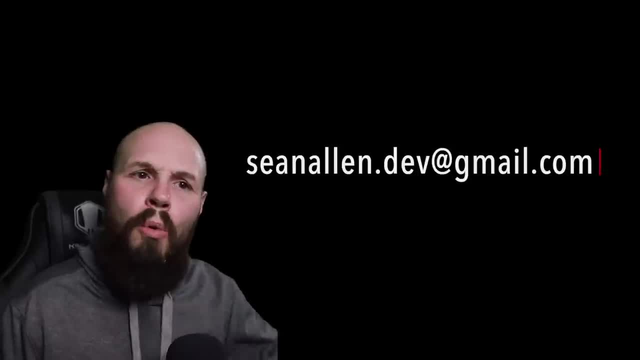 So please let me know what did you enjoy about the course, Like, what should I do more of? And, more importantly, I think, like this is the feedback that I actually look forward to- is the bad stuff, Like: what did you think was too confusing? 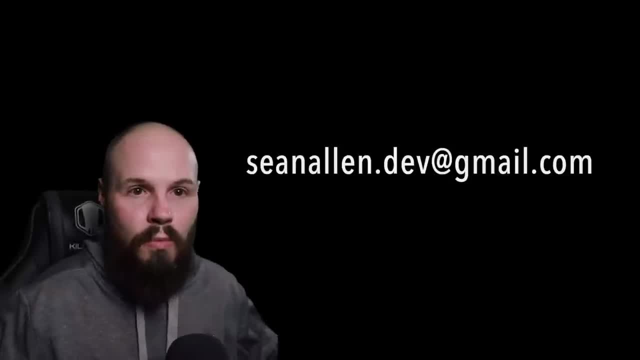 Do you think I explained something in a wrong way? Just what did you not like about the course? Like to be quite honest. even though a lot of people don't like sending that email, those are the ones I like getting because that is how I improve by fixing all those things. 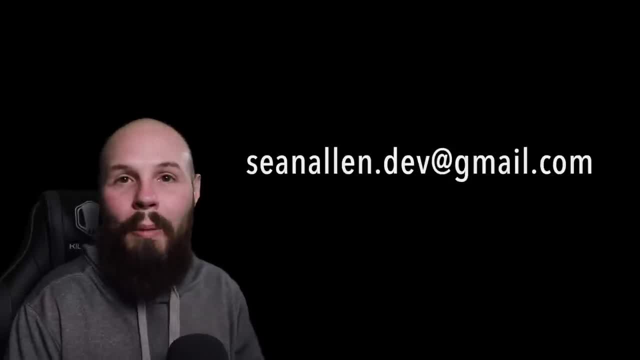 So, please, I would love to hear your feedback And then also, while my email is up there, if you did enjoy the course and you wanna leave a testimonial that I can post on a page so future potential students when they're looking at the course. 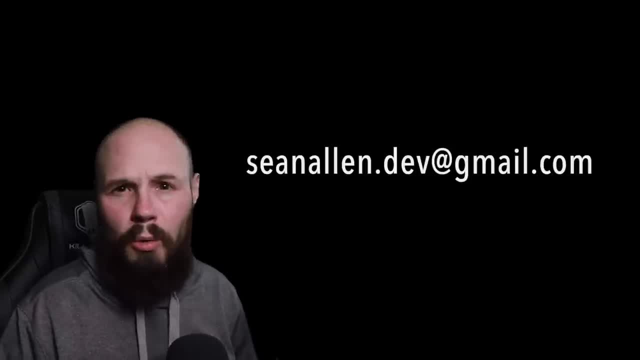 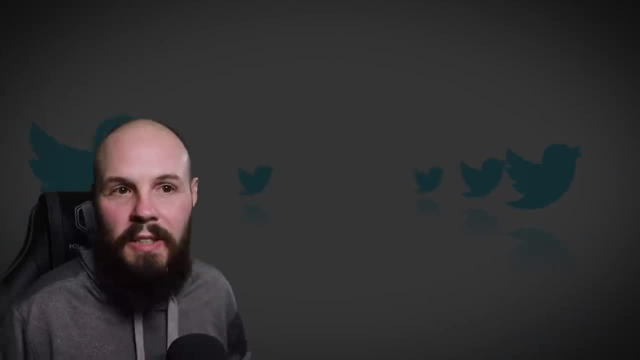 they can see. let me know Or just email me a real short blurb, like two sentences, and I will put it up there as testimonials on the course. And then, finally, if you enjoyed yourself while you were taking this, please tweet about it, share your experience. 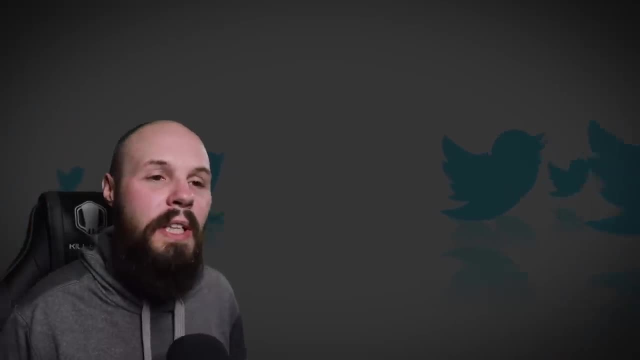 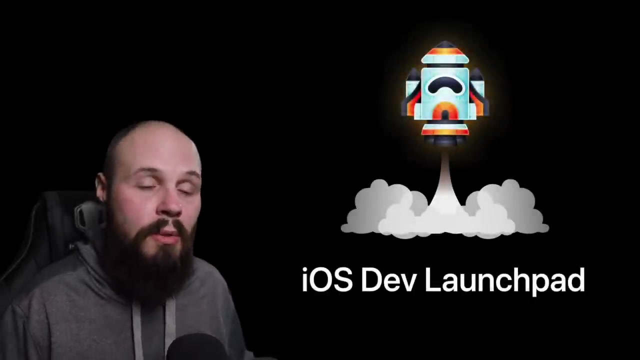 talk about what you liked about it, I'm happy to jump in there, retweet it. It just really helps spread the word and get my courses out there and more people exposed to again what I'm trying to build here with some of the best courses in the world. 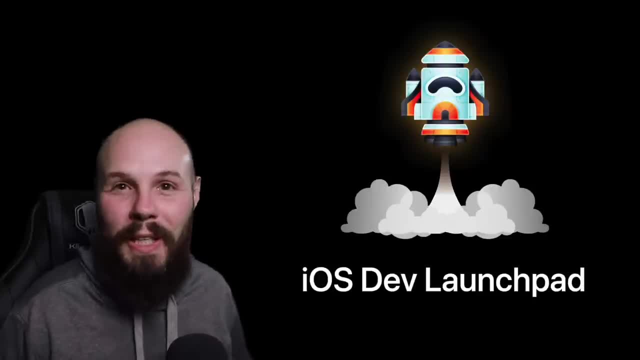 That's the goal. I'm not claiming that I'm there yet, So I hope I don't get emails like. you're nowhere near that, Like I know. that's just the long-term goal. We're trying to get better. But again, thank you so much. 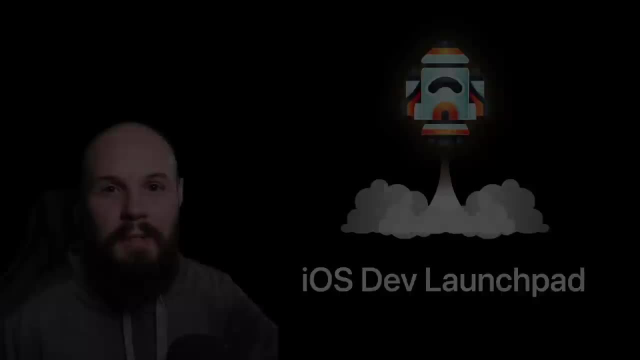 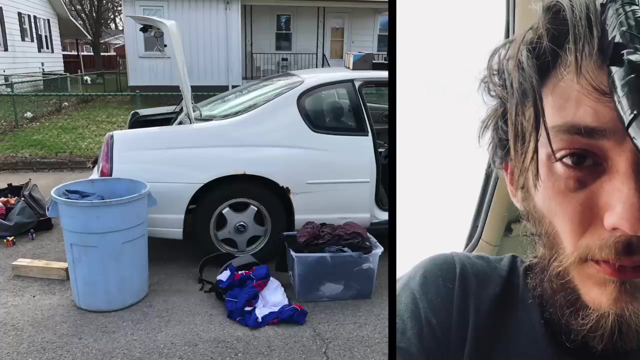 for coming on this journey with me And I really hope I get to see you in future courses. Ezra Black was homeless in a car in a McDonald's parking lot, stealing wifi, learning how to code, And now here he is, full-time developer. 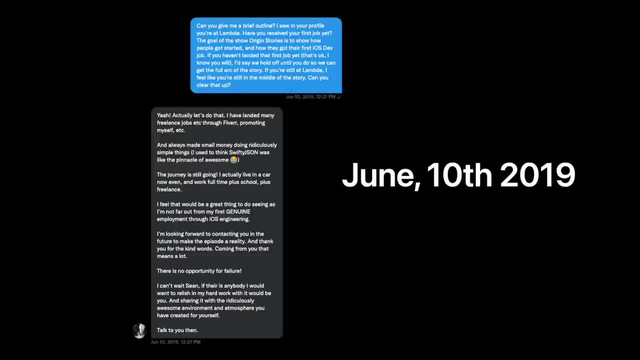 making well into the six figures. He reached out to me about two years ago and told me the beginning of his story, you know, before he got that job and I told him: no, no, we'll have you on the channel. You know what? 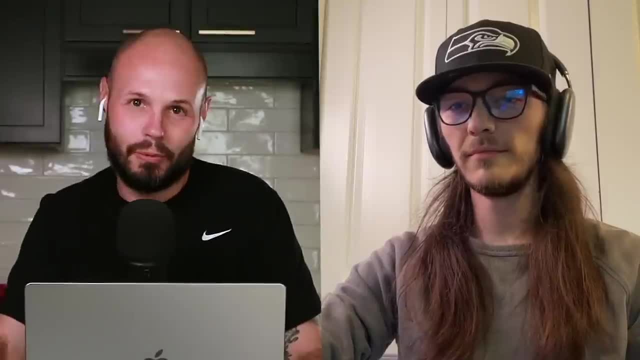 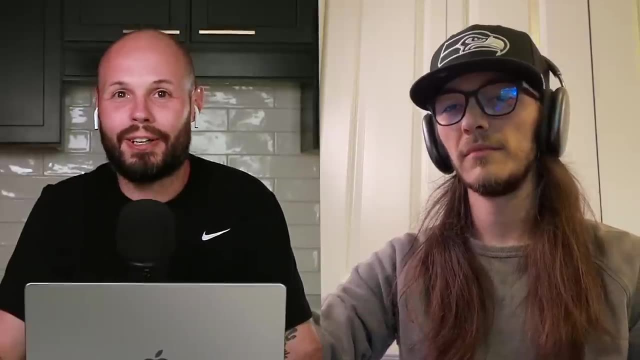 Let your story finish. Well, here we are, about two years later. Welcome to the channel, Ezra, Happy to have you. I want to throw it to you right away Because, again, what stuck out to me about your story was: in a car, in McDonald's, stealing wifi. 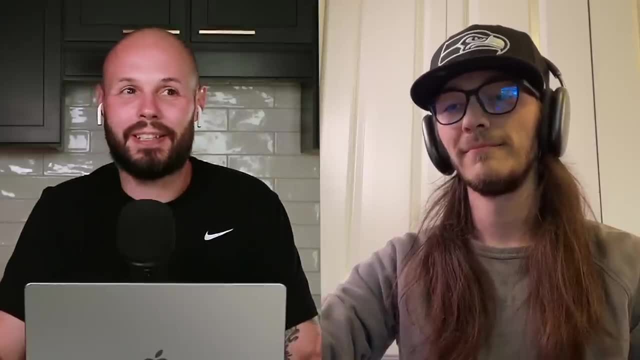 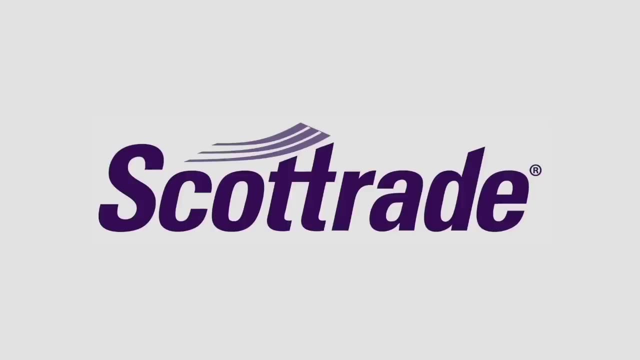 watching YouTube videos learning how to code. So just how'd you get there? And yeah, just start talking about that. Yeah, I ended up getting into the position due to Scott Trade. I was working for the Scott Trade investment firm. I was doing security work for them. 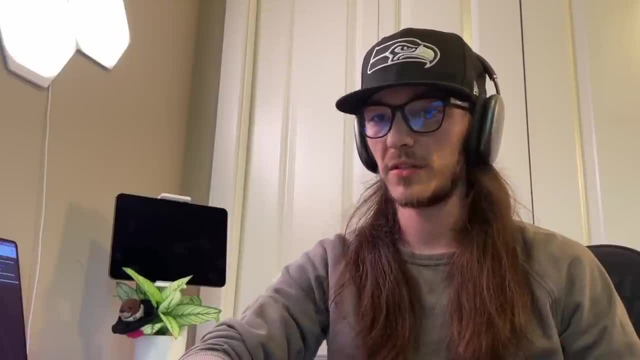 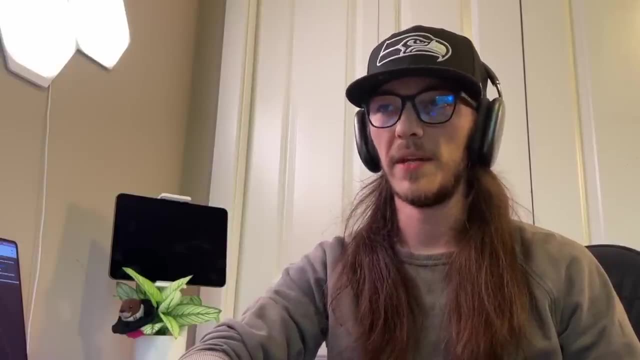 through Allied Universal and working in their technology fields. just, you know, being the guard there And that got me really interested in the technologies and getting to be around. you know the kind of environments that technology brings. And then Scott Trade closed in 2017.. 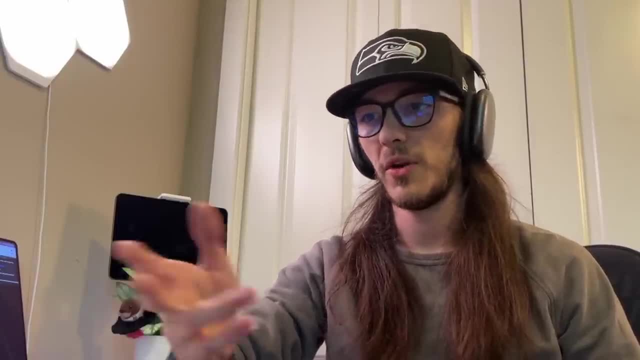 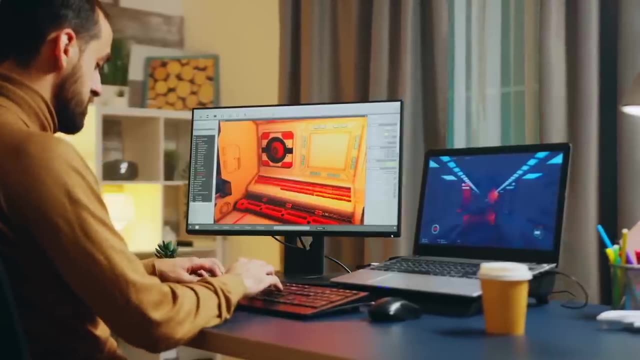 And whenever they closed, I didn't have a backup. So I found myself, you know, dealing with a strenuous situation of money and income: working like small contract jobs, doing things like that, and messing around with coding Like I was building like little video games on Unity. 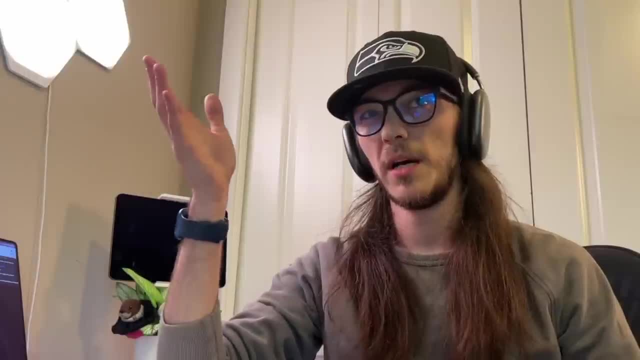 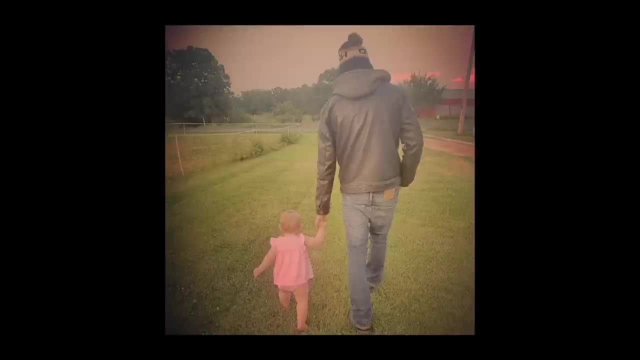 and stuff like that, which I really enjoyed, but it wasn't really aggressively in my mind to be something that I really wanted to focus on. Once the mother and my child, though, separated from me, I didn't have nowhere else to go. 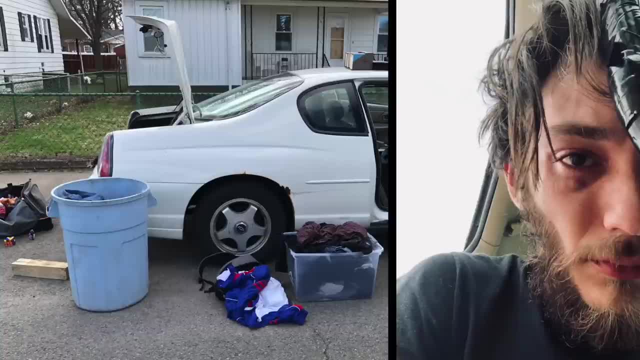 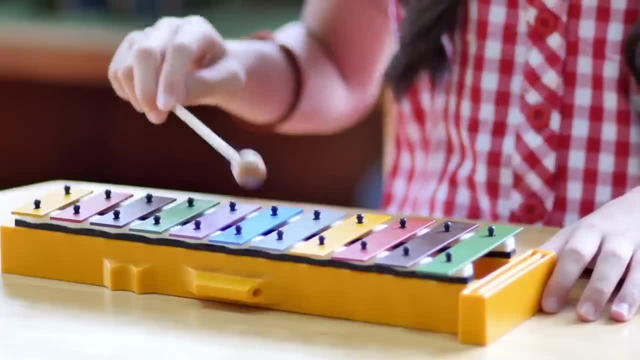 And I started living in my car. That's whenever it really started to accelerate. I started doing, you know, little teeny courses and things like that, And I built a xylophone app for my daughter when I was younger. So that's kind of what hit it off, was this xylophone app. 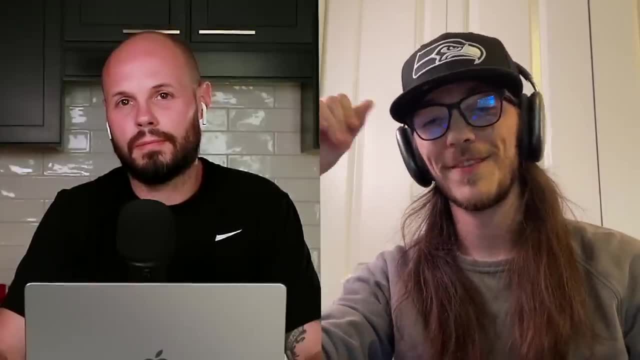 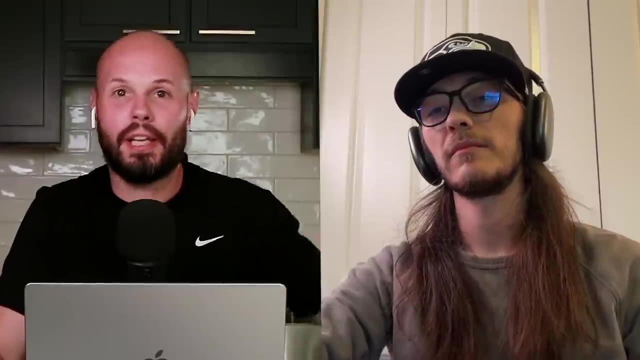 that I wanted to build for my daughter, So she wouldn't use my phone no more. And we find ourselves here now. So was it always iOS? Were you? I guess, Yeah. how did you end up in iOS and not Android or web? 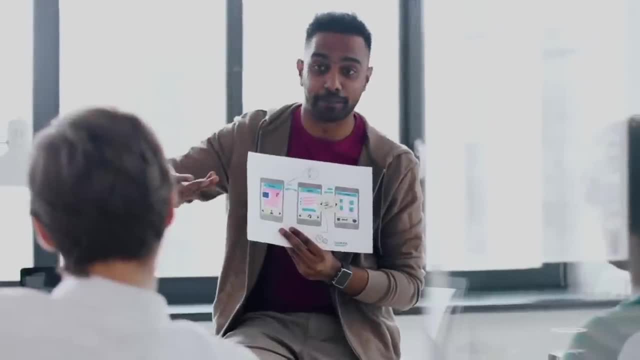 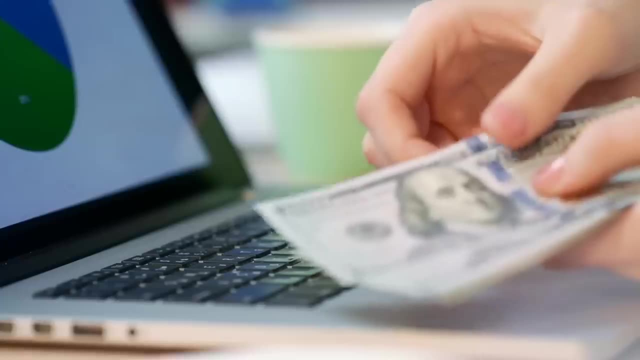 Good question. So, honestly, I kind of did a little bit of research. I wanted to do mobile development because it was the only device I had, So I didn't have nothing else with me to actually code with. but I looked at how much they make. 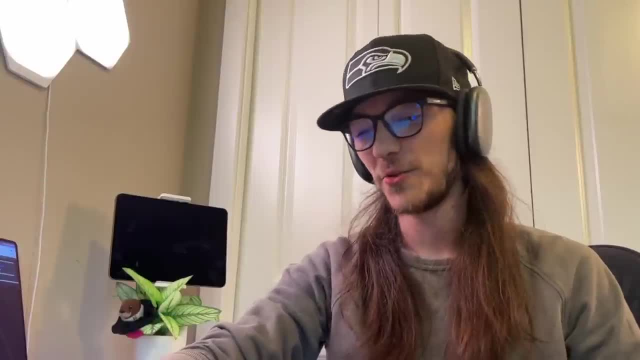 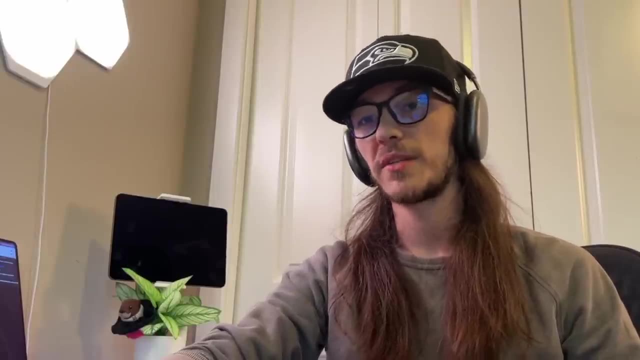 So I'm completely. you know, check the field, I checked Glassdoor, I checked all that other stuff. I just wanted to be able to make enough to really support my family and be able to support myself as well. So iOS just ended up being the smarter choice. So talk about iOS. 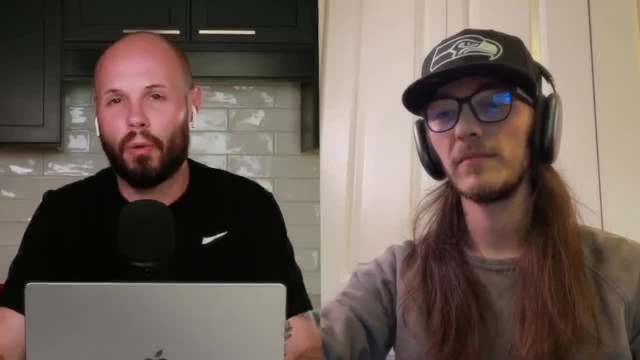 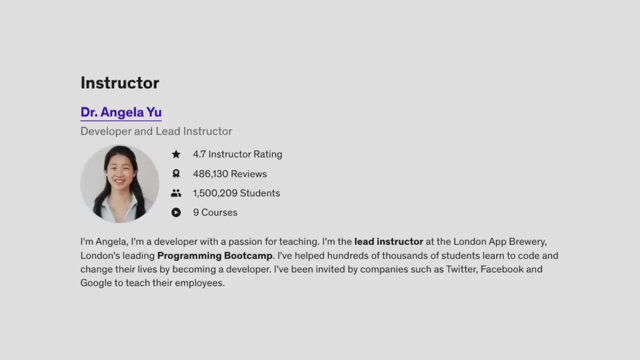 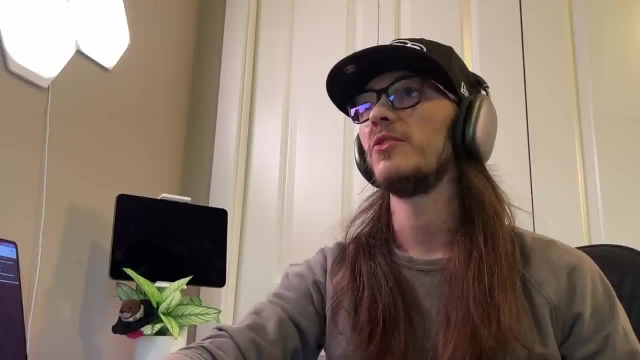 and it would buffer all the time. Yeah, definitely. So I started with Angela U courses Eventually led into your courses, just searching for things through you know needs that I had for hers and that actually led into needing better Wi-Fi. So I was doing the McDonald's needs. 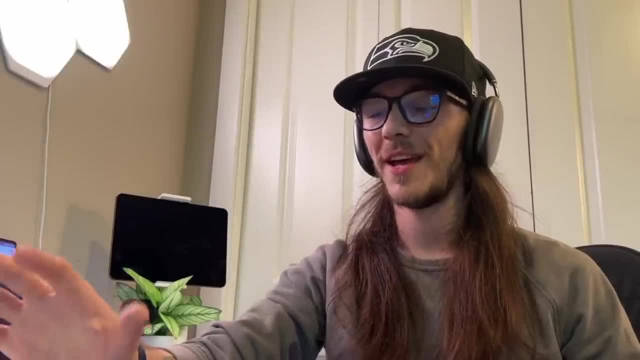 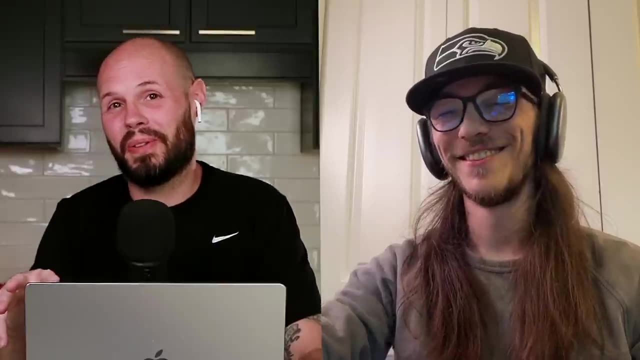 They were letting me use it three or four hours out of the day, and then I'd kind of sit in my car and get close to the building, you know. so they didn't like that too much. I ended up making so they knew you were using it though. 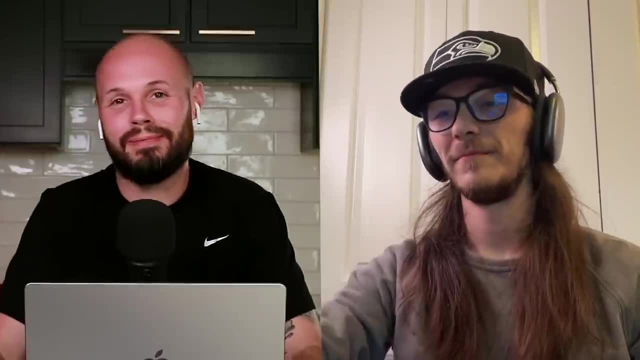 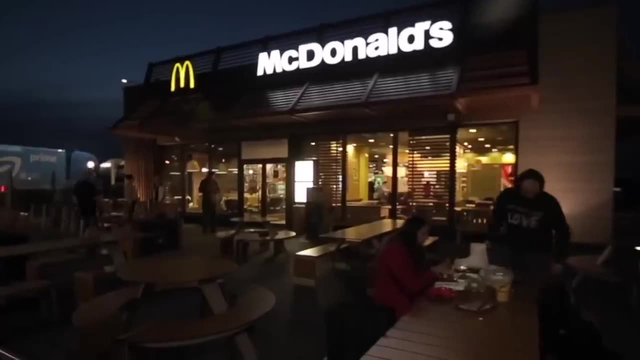 They weren't. you weren't like you know, yeah about it. They knew what was going on, except at nighttime. So eventually, though, they did start cutting their Wi-Fi on me, because I had like two or three people out there that started figuring it out. 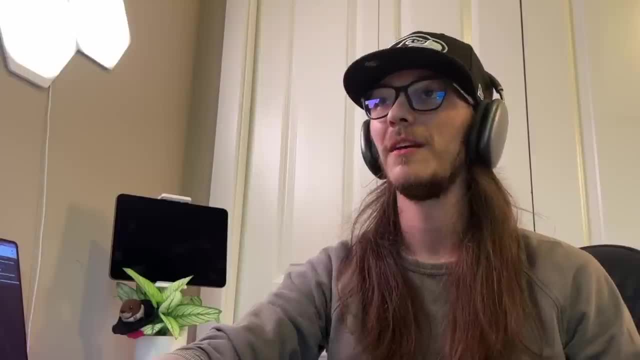 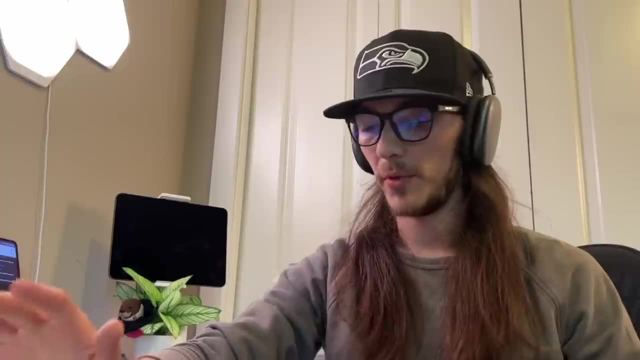 So there was like a lot of people huddling around the building and using the Wi-Fi and everything. I had a friend, though, that went to the Community College right across the street, and I eventually convinced him, like I was like, hey, you know, like I really want to get into this coding. 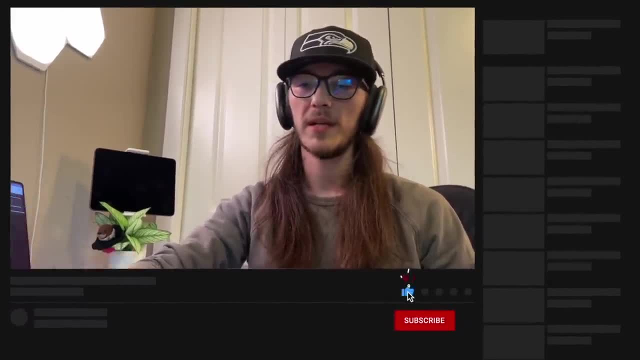 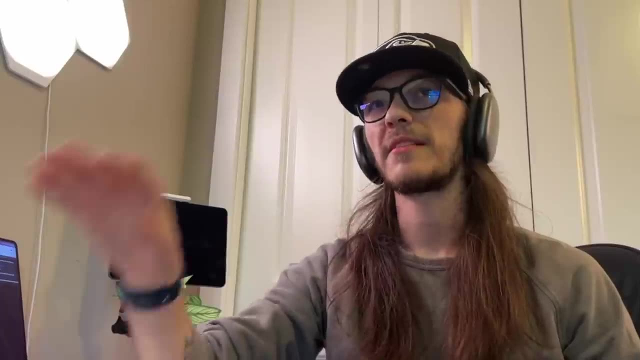 I'm trying real hard. I showed him some of the example tutorial apps I was building and he was down for letting me use his login credentials at the Community College, So I was able to use that Wi-Fi for the last stint before I finally signed up. 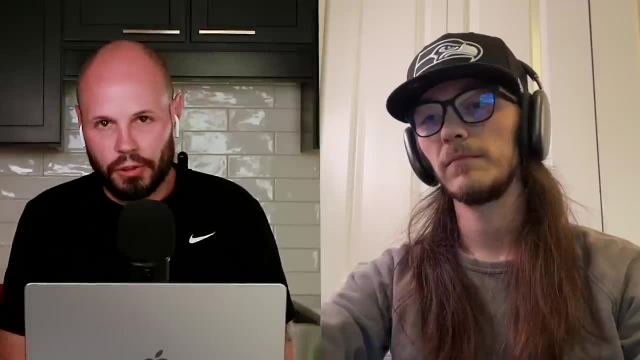 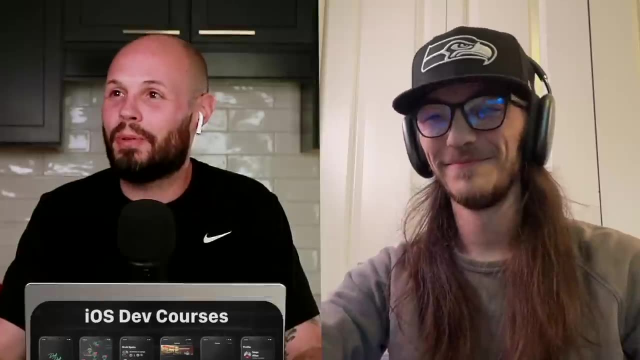 for the coding school that I went to. back to the YouTube a little bit He said, Angela, you courses my courses, I. the reason I want to go to this is not to brag about my courses, but I I like to tell people that, like, YouTube is so powerful right. 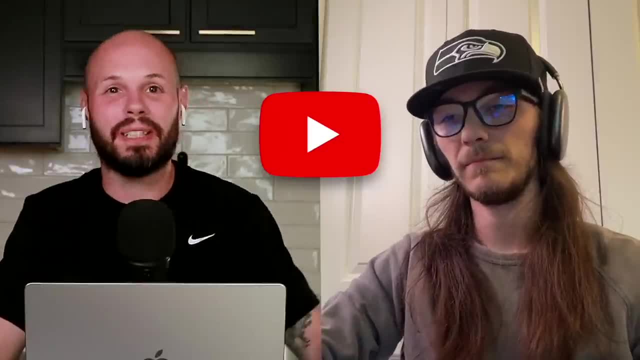 I call it YouTube University. You know a lot of people think you need the computer science degree and all that stuff. It's like man, everything is is for free on YouTube, or even the courses are relatively cheap when you compare it to. you know. 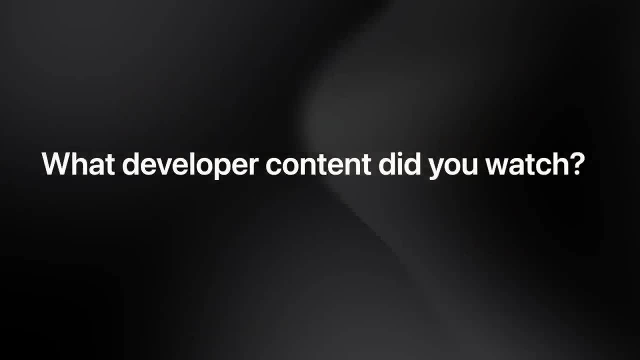 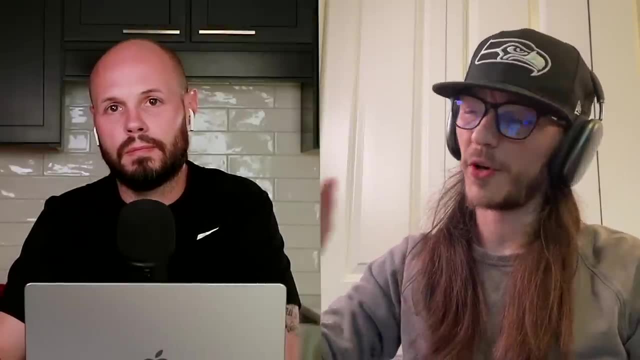 going to school for it. So I guess maybe dive into more about what videos you were watching, as far as like tutorials or even like motivational videos to inspire you. Like, what were you watching? you had a video before your courses- I speak about those. you had a video talking about how to be, how you became. 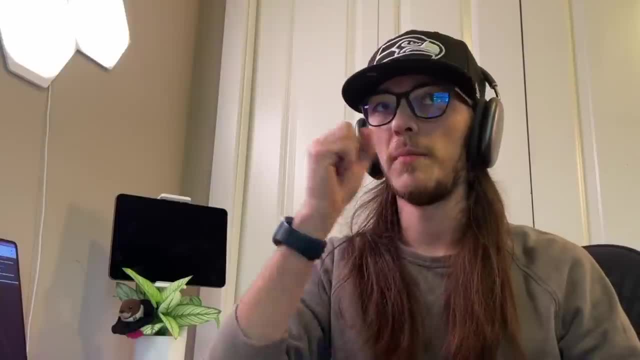 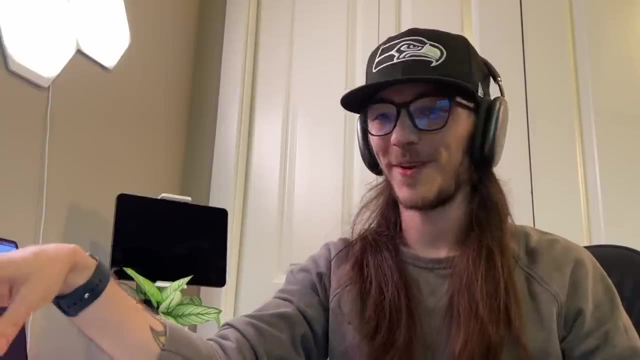 an iOS engineer in seven months and that really opened my eyes and I can remember I was actually sitting in a McDonald's with like four old people next to me and they were talking about. they were talking about funny things and the guy next to me I can remember he even told me. 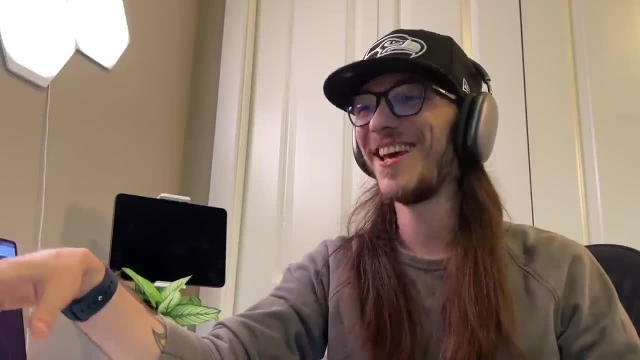 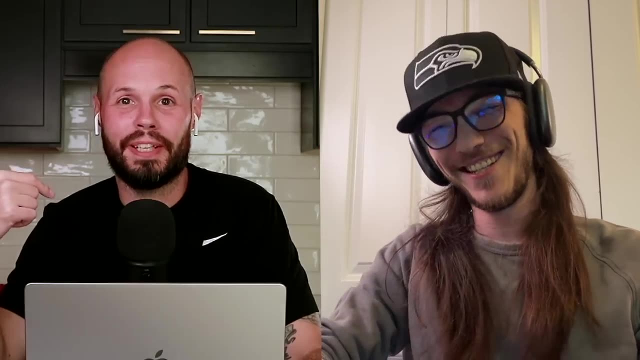 He goes, that guy's telling you a whole bunch of malarkey. That's what he said. He was like you need to go out and get a job, you know, and everything else like that, and get off your laptop. and I was just laughing because I was like you saying about me on the on the video. 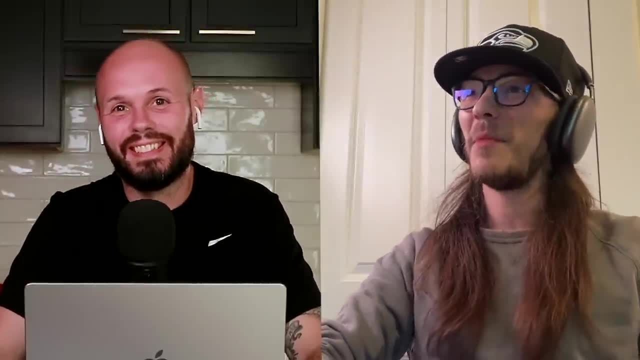 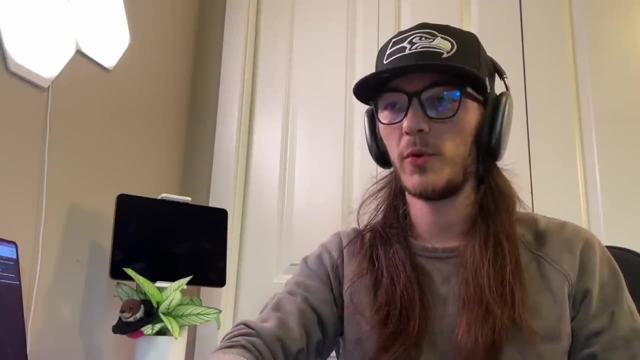 It was like all you're just listening to, you know some older man and yeah, but I'm definitely just general motivational videos and stuff like that, But within coding world, it was definitely you, of course, and Paul, so Paul was a really big inspiration. 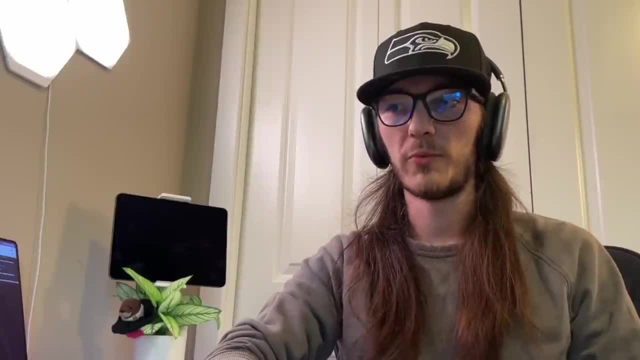 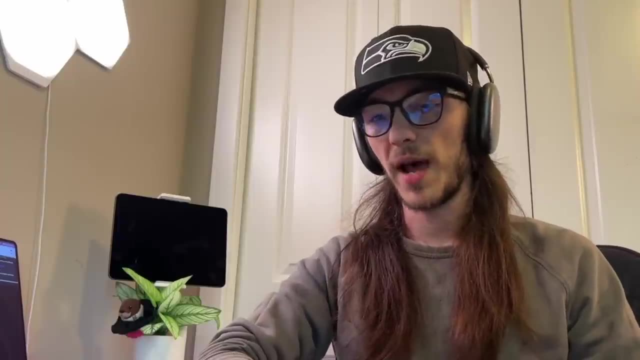 as well, and a really big help. just having the information out. there was what really hit it off for me. realizing that all these different people that were already really far into the field or, you know, really established, were providing these kind of resources and really making it seem like it was a transparent path was what really led me. 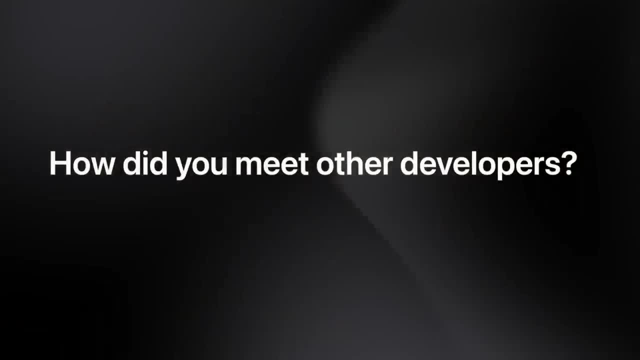 on to feeling like I could, like, hey, I could do this. you know how did you handle, like meeting other developers- right, Because obviously it's probably not too many of them sitting in a McDonald's parking lot- Like, how did you go about, you know? 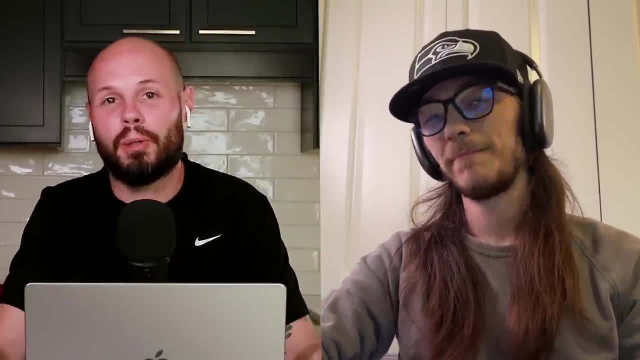 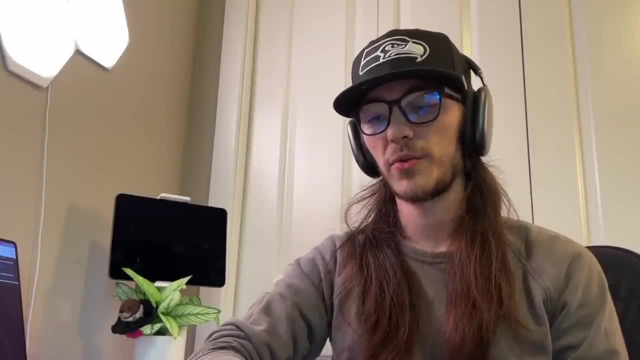 because you probably get stuck watching these tutorials or courses and you need to reach out for help. So how did you go about that? So it started with Twitter. Angela talks about you know, doing the courses And everything, and, as well as you, talking about how you do social medias. 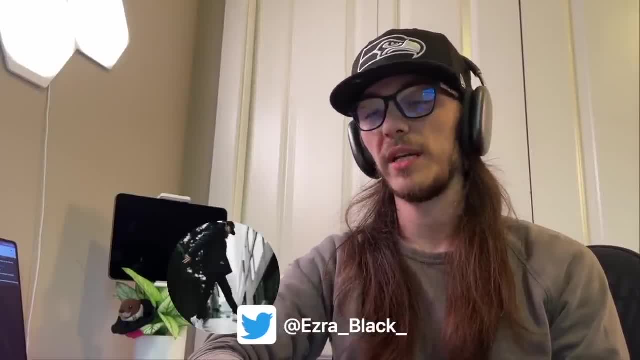 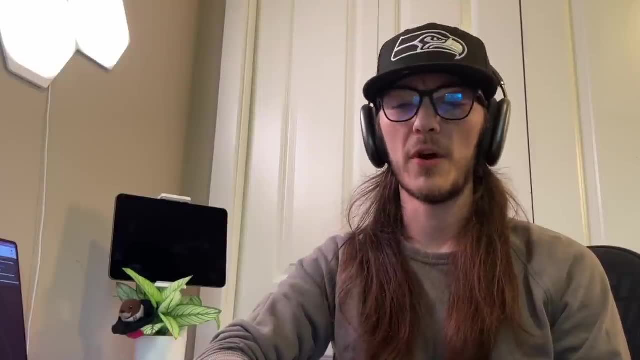 I had a Twitter before, already for years. So I was like, well, maybe I should just really get into this. So I focused a lot on building my Twitter and following different iOS engineers. I kind of just stalked everybody's followers, you know, and went through and found every iOS engineer I could find. 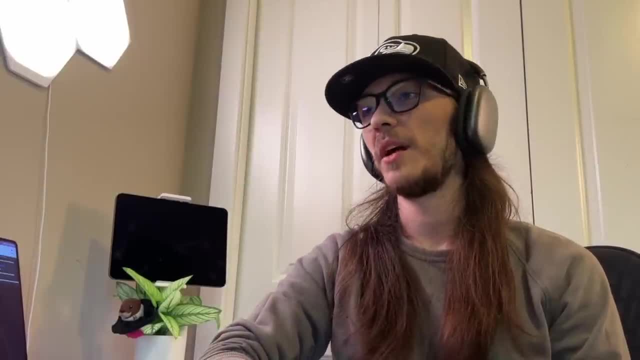 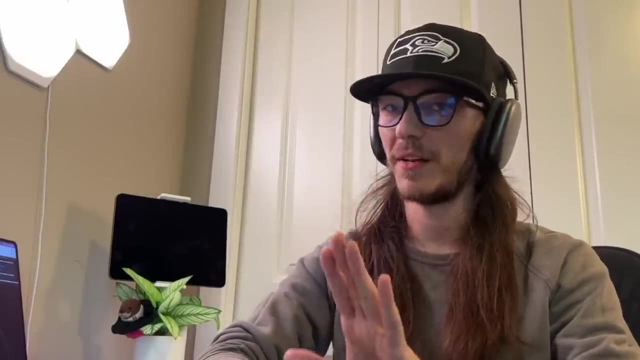 you know, shoving random questions down people's throats that they probably don't want to hear A lot of. it definitely was just getting into the internet side of things because I got lucky. Well, I guess I shouldn't say lucky, Let's not call this lucky. but COVID happened. 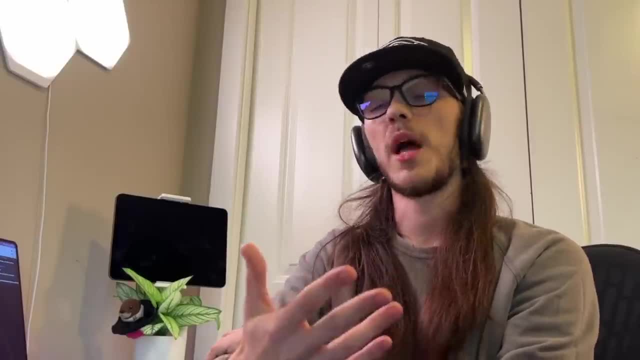 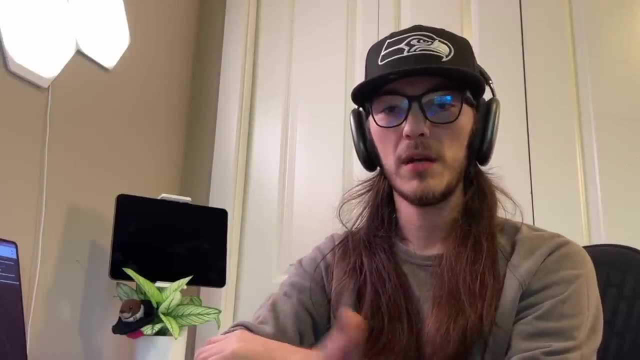 So I was homeless and whenever COVID occurred, everything went online. and because everything went online, I was able to get a lot more of a quality of interaction with the community, which is what really hyper accelerated and, like, propelled it forward. You said those key words. 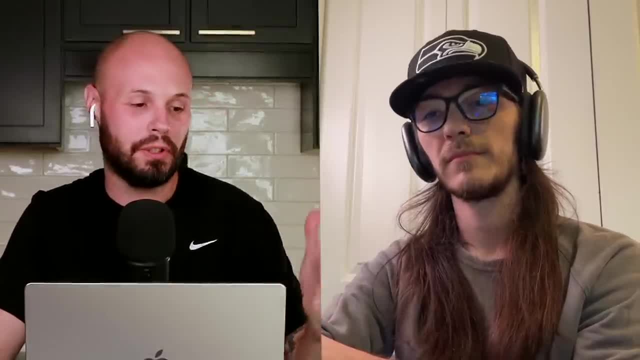 I was going to ask you about. you said, propelled it forward. I was going to ask, like, how did you? you know you're sitting in the McDonald's parking lot- and then, like you said, you eventually got to do the community college Wi-Fi, What was kind of like the the big break. 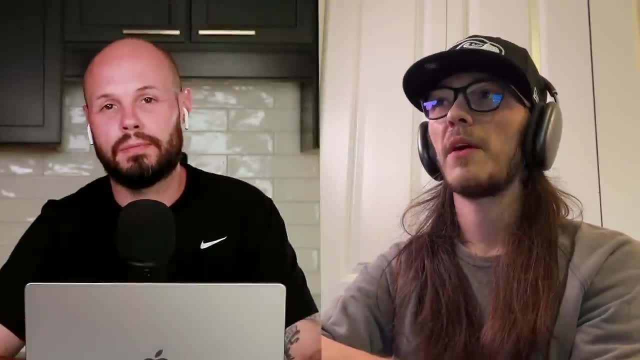 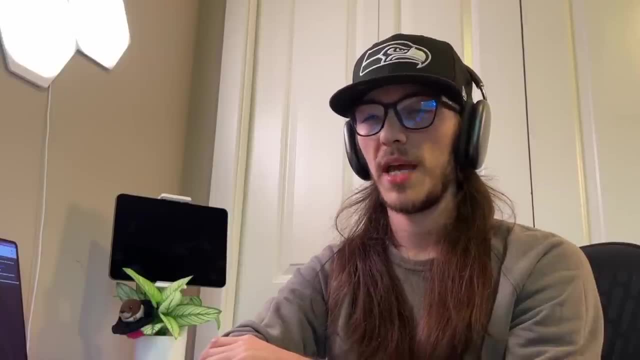 or at least the start of the big break that started you forward. I think my first big break was getting into lambda, because I started the lambda boot camp and they have like a six-month, nine-month course and getting accepted into that real quick. You said it was a big break. 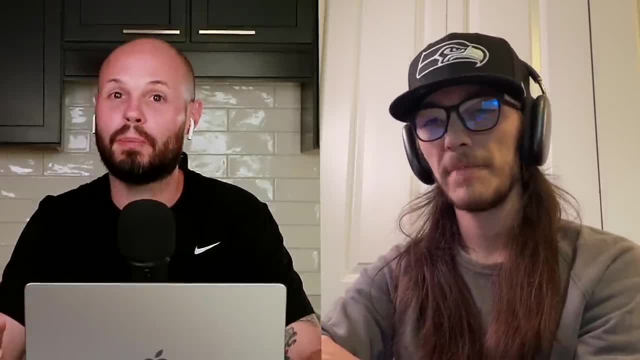 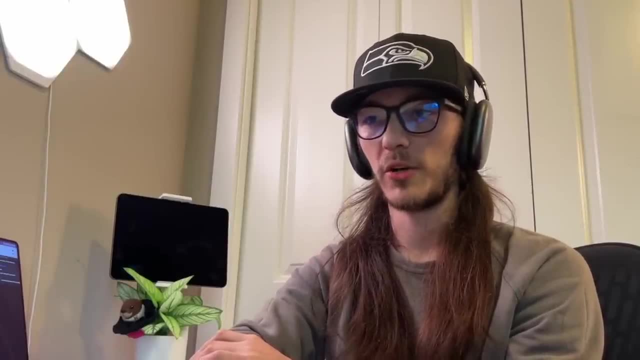 Was there a stringent application process? Like I, like, how do I? was it a big break just to get in? Well, I've never really accomplished too much in my life academically at the time and they did have like a huge like beginner course. 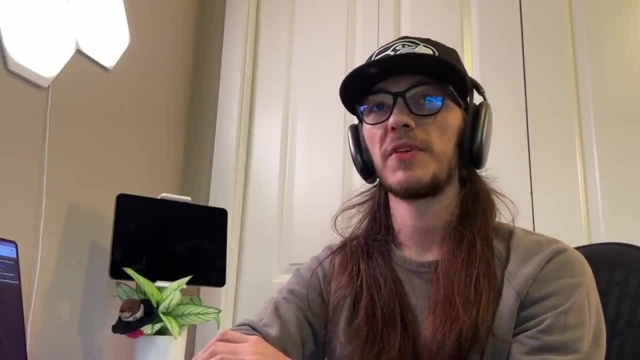 that you had to do. at the time I thought it was a lot bigger than what it was, but it was the first thing that I ever did and like had a reflection on like: hey, this is something that you're valid with, this is something that you can do. 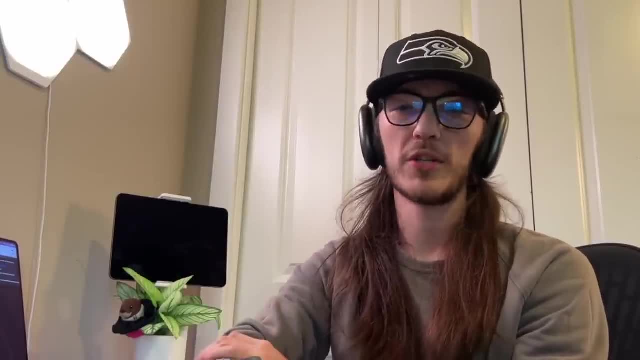 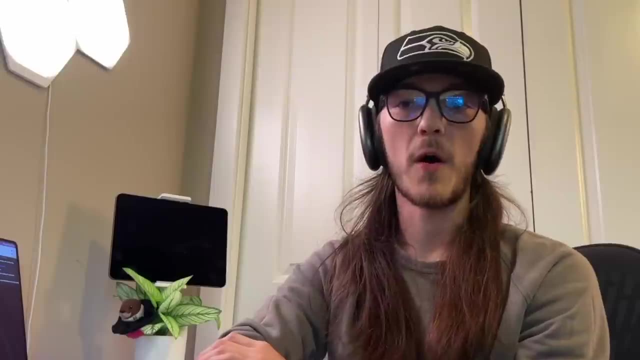 and getting done with that crash course. In the beginning They had like 60 iOS questions, you know, in like a basic app thing you had to do. accomplishing that and being told like hey, you know we're going to accept you. and knowing that I was sleeping in my car. 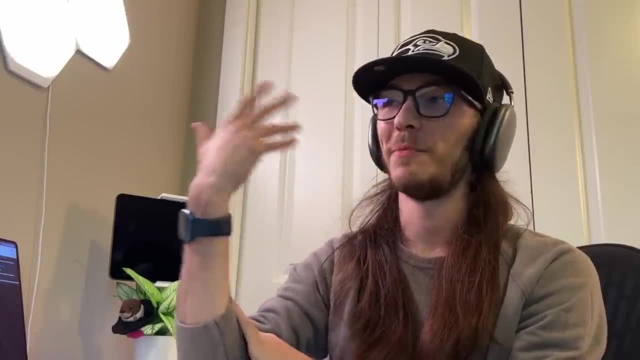 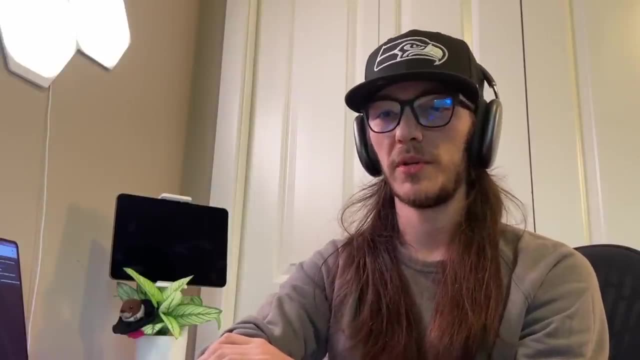 and then seeing all the other people that were there. you know, hey, I'm in my car and these people, you know, have beautiful desks already and setups and you know all the gear and everything and I'm on equal level with them. So that was really like a. I can do these things even in a more stringent environment. 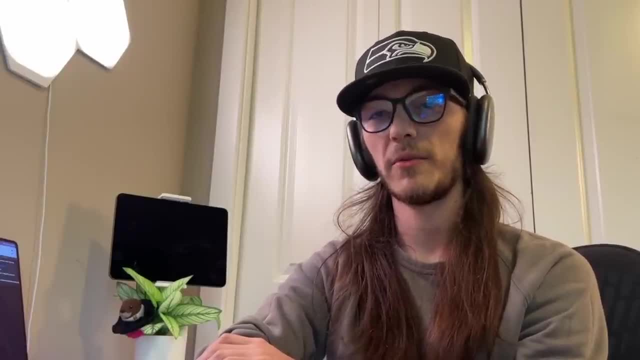 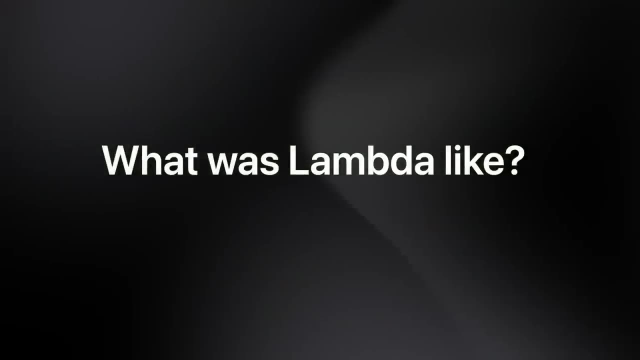 and because of that, it made me feel like I was like: hey, you know, this is something I can really do, This is something that I'm good at, You know, it was the, the validation outside of myself. So you, you're into lambda talk about the boot camp process. 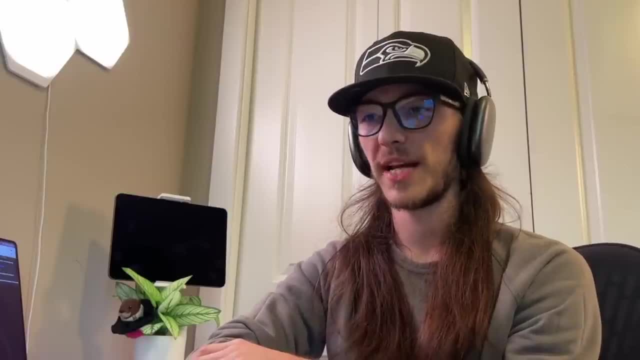 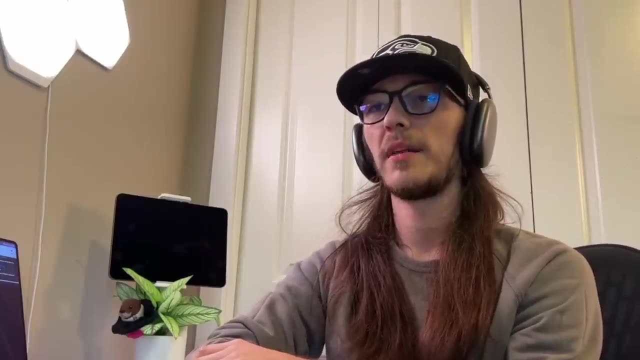 So that's what's really interesting, as well as that. once lambda started- That's whenever covid started getting really big- I started interacting with different people in the community and I ended up meeting a girl named Zoe through the internet that I ended up starting dating. 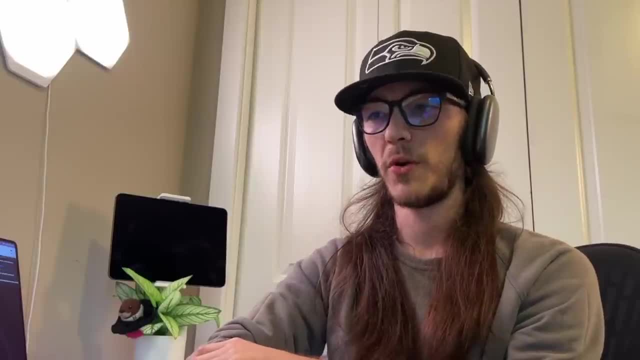 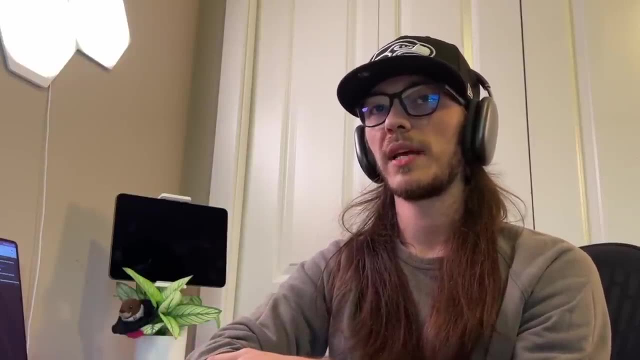 I think it was beginning of 2020.. That was whenever, like, the boot camp was starting to ramp up and everything. So I had a little bit more comfortability once it actually started to ramp up. but the experience in lambda in general and like the coding experience, was pretty solid. 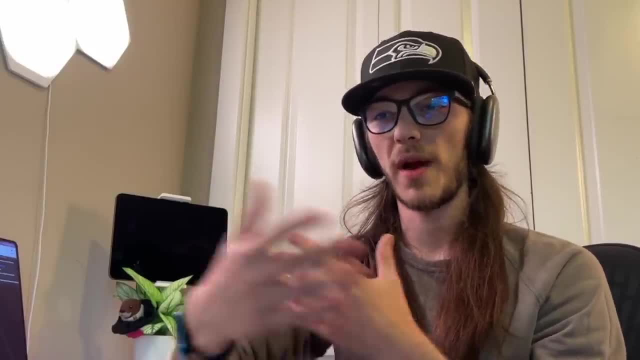 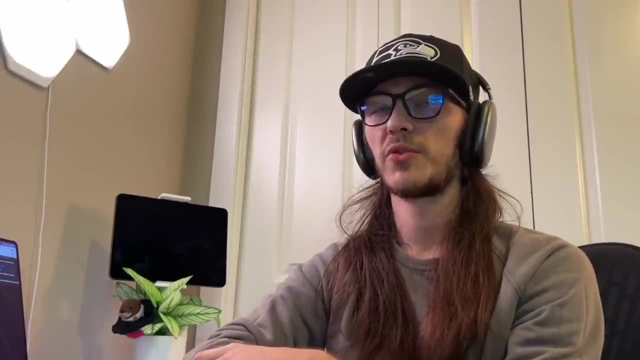 I'm not going to lie, like after I got out and got to experience like the real environment. They did a pretty okay job at like getting you the blanket understanding of things and having a good syllabus, but the school was just not accommodating for how I learn. 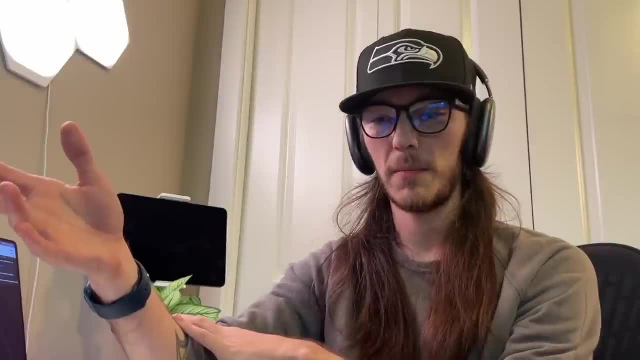 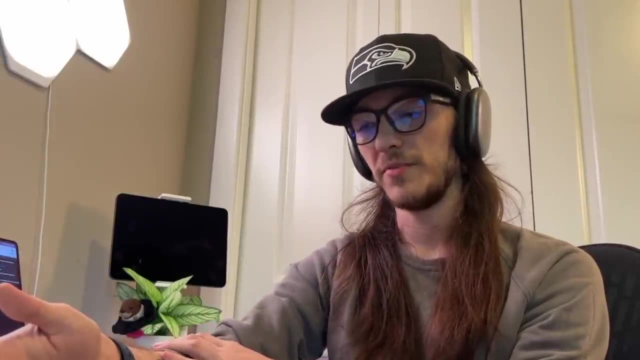 and the fact that I was just getting out of a situation that I got out of and dealing with, you know, rehabilitating myself into normality. and then, on top of it, covid happening, moving. you know, I moved from St Louis area to Springfield to be around Zoe and starting. 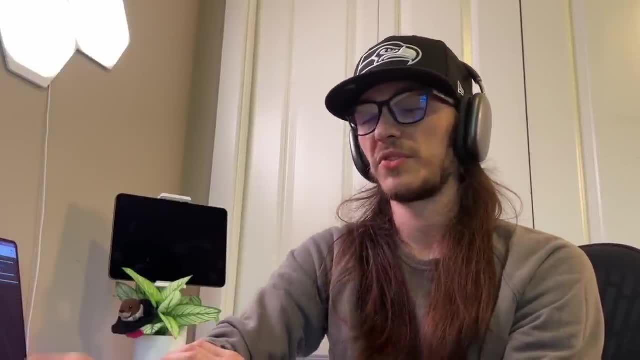 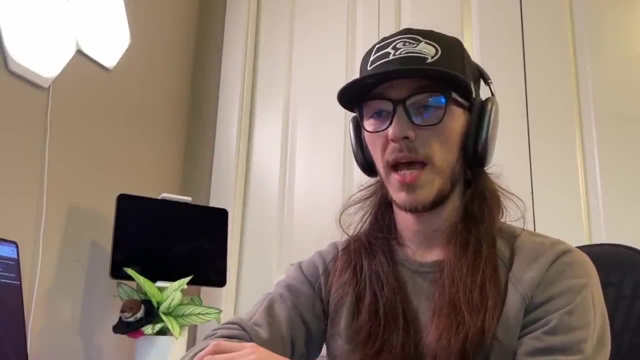 I am to hardcore in general- made it just. it was something I couldn't accommodate myself to, no more. So I kind of just took what I knew and then what was left in the syllabus and kind of went wild on the internet. I dropped out of the school, did the hacking with Swift. 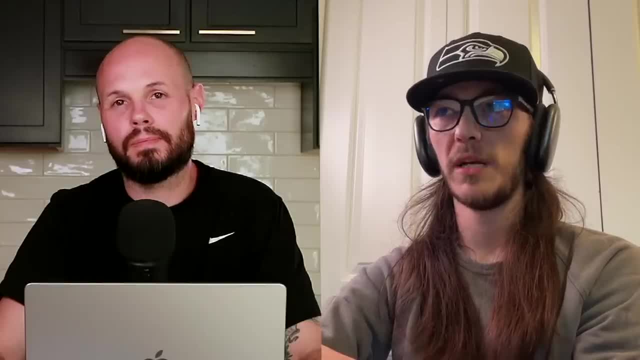 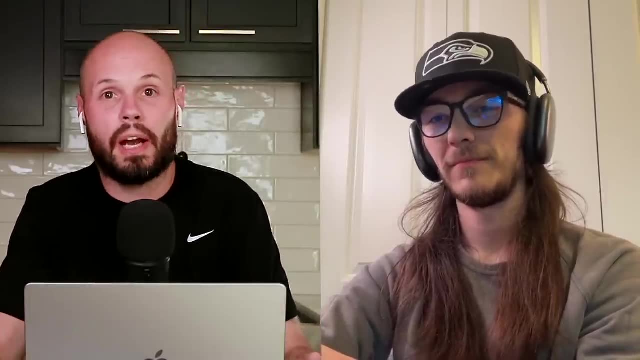 you know, just grinded out that last little bit and started doing interviews. So it sounds like that wasn't a setback, because I would have thought, you know, quitting or leaving the boot camp would have, you know, set you back, because we just talked about how that was such a like big accomplishment getting in. 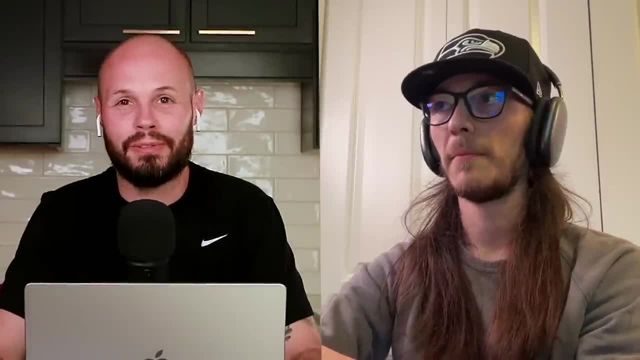 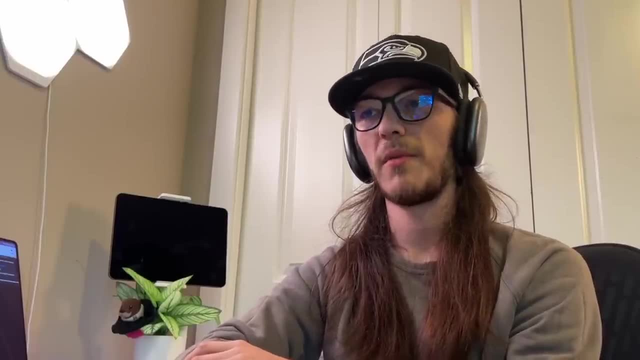 But it sounds like you just kind of kept it moving, Didn't you? Yeah, not too far. And what I realized was that I wasn't there to get the piece of paper. I was there to learn. once I knew I felt like I was comfortable. 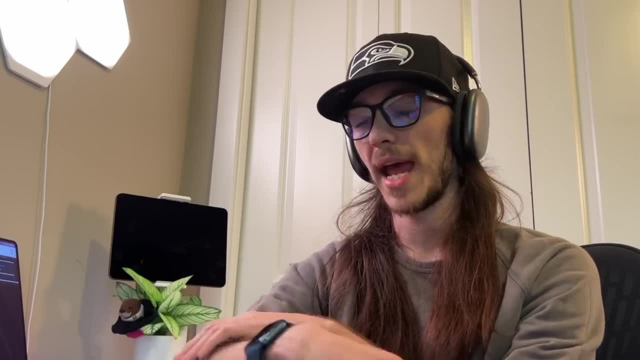 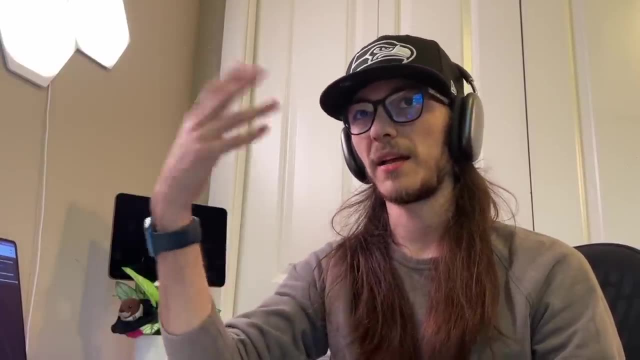 and strong in my understanding of what I can and can't do with coding and how you teach yourself. I just hit the races, You know. I was able to take the syllabus and realize like I was like hey, I got like four more months left of this if I drop out now. 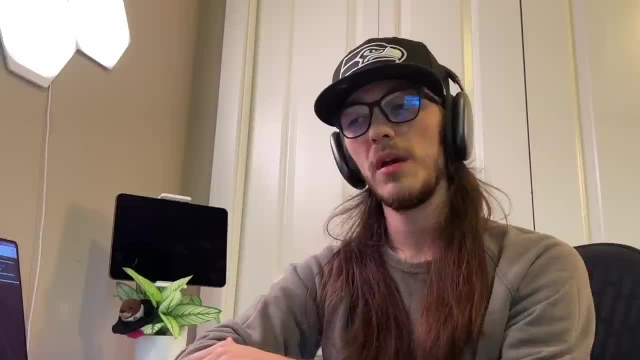 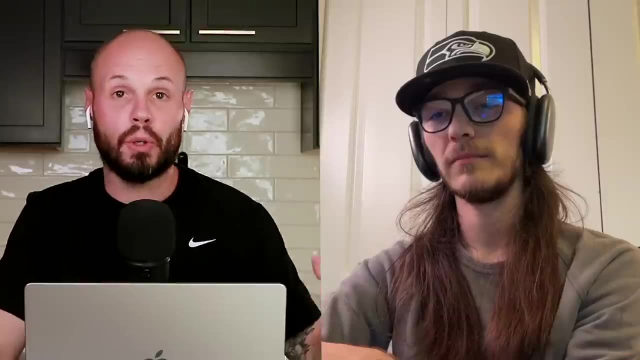 I can hyper accelerate myself through this whole situation is going on with covid and have a potential chance to, you know, just break out of this tutorial chaos. you know, after the boot camp you started going on interviews and I know one of the questions I get asked all the time because you know. 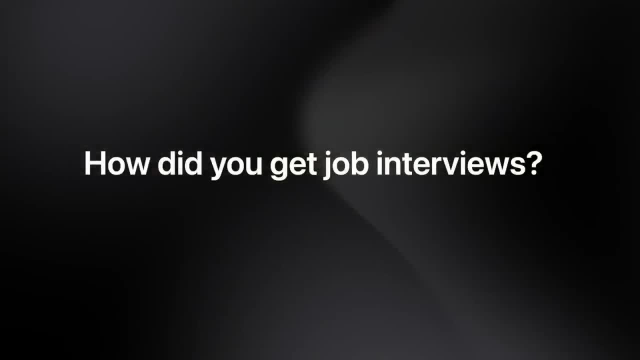 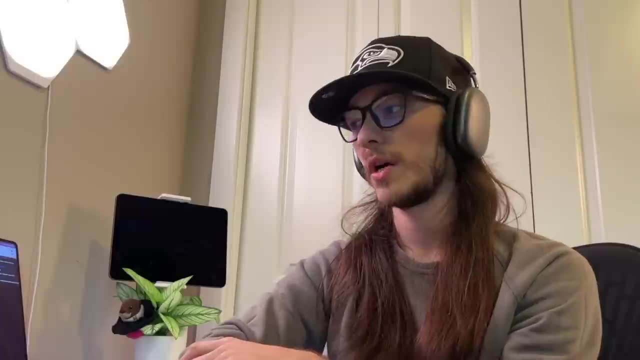 most of my audience is trying to get that first job is: how do you even get these interviews? So talk through, like, how you got these interviews and how that led to maybe even more interviews. Yeah, so I kind of wanted to stand out. That's an interesting question. 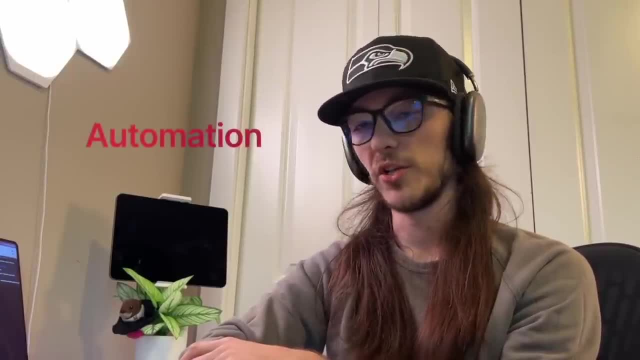 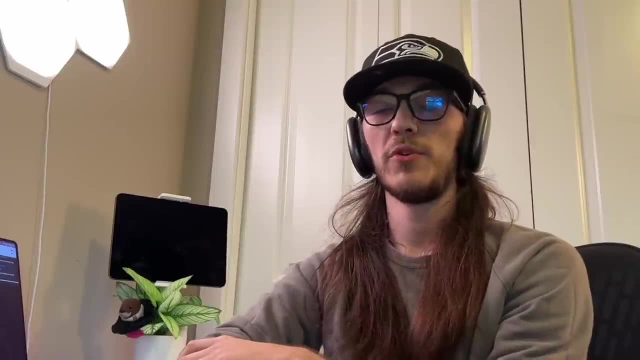 I started getting really interested in my own fields and everything which was automation and augmented reality, So I kind of fiddled with both of those to stand out. since I didn't have a degree or nothing. What I started doing was I would do man-in-the-middle proxy attacks on their application. 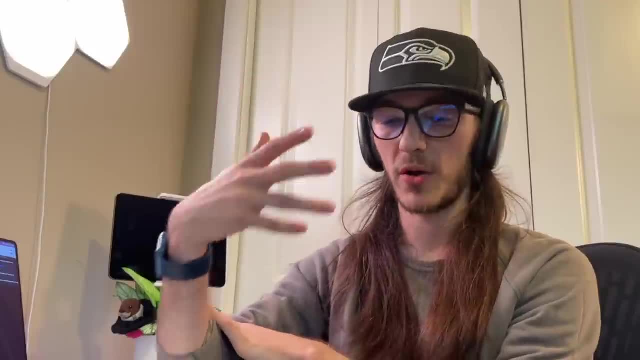 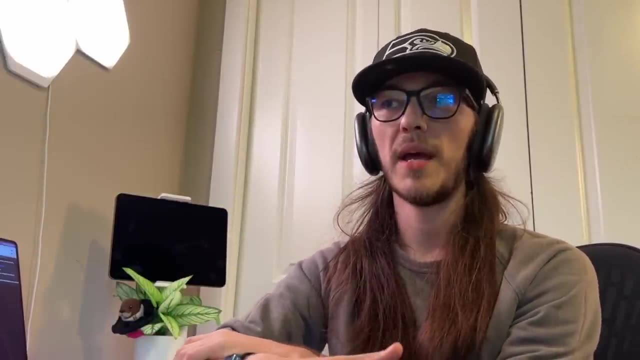 and then I would go through all their JSON- you know everything that gets everything that goes out publicly on the phone- and I would structure everything and tell them what tools they're using and everything else like that, Instead of just having you know, like my resume. 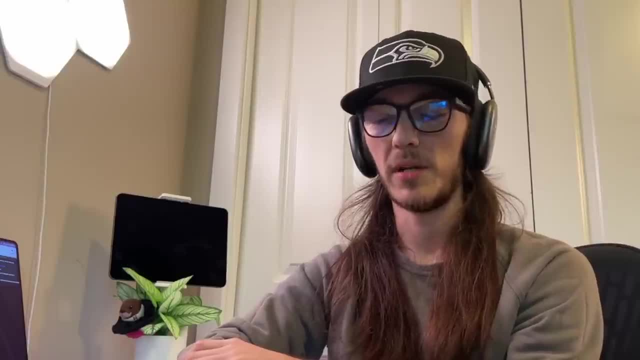 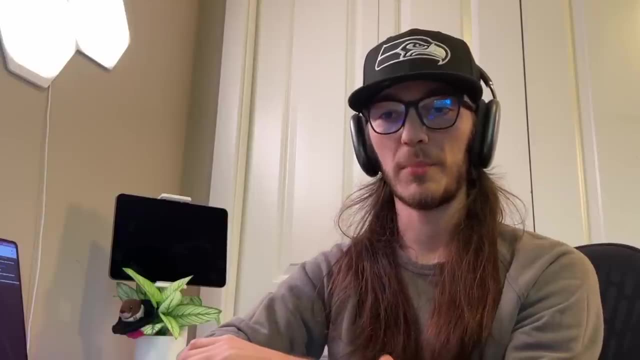 I would give them a cover letter, which was a diagnosis of their application, or, you know, like any things I might have found, or like the technologies that they use and why they interest me. you know just the journey of exploring their application and telling them I enjoyed. 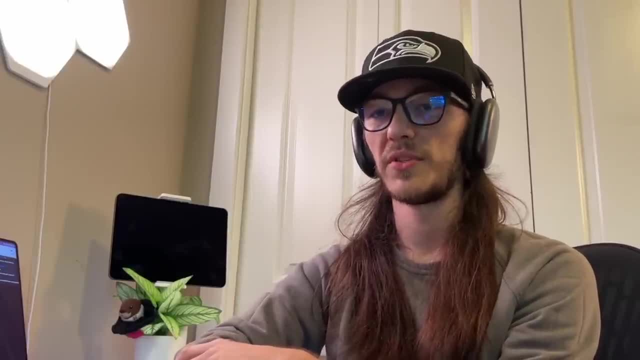 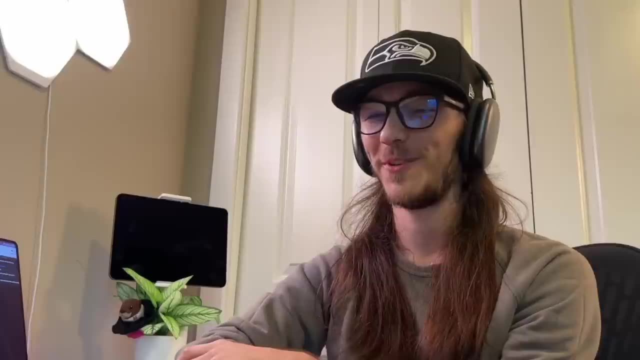 you know the technologies and what they're using. that usually really was a standout thing. I got so many interviews that way. you know I didn't get the job, But I definitely got the interview. just, you know, somebody being all like who in the world is this guy? 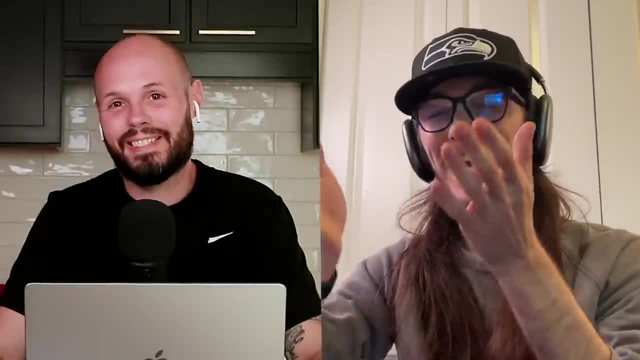 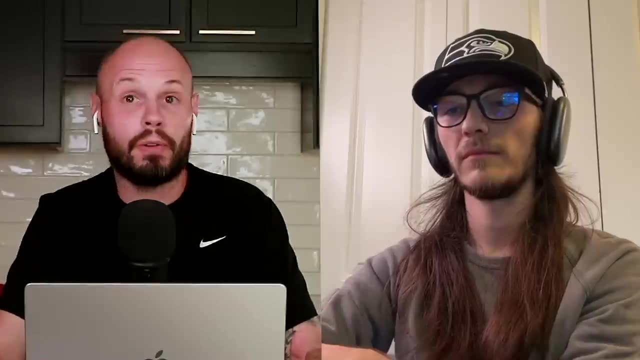 So it was definitely a good idea. Just just try to stand out a little bit, That's it. I just kind of say that about my YouTube channel, my Twitter and the brand and everything like that. Like, I can get an interview pretty much everywhere, whether I get the job or not. 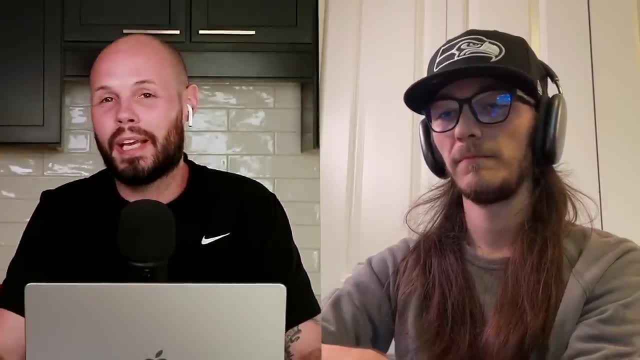 Well, that's up to me, right. But all you can ask for is, like, the chance. do whatever you can to stand out to get that chance. And then you know, the interview is a whole nother story, but at least you got the chance. Yeah, you know. 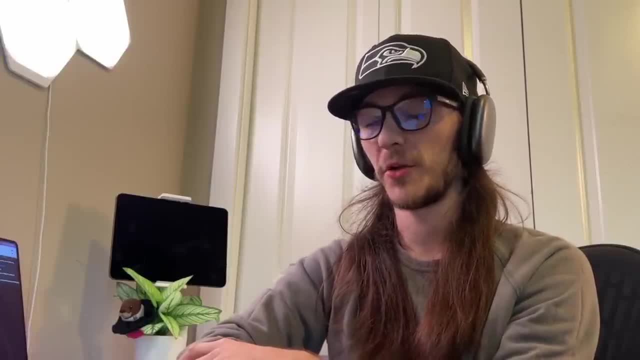 I've seen people in interviews come in and you know they just have that amount of charisma that they can understand things. or you know you go into jobs and you don't understand the frameworks that they are using. People can teach people how to code. 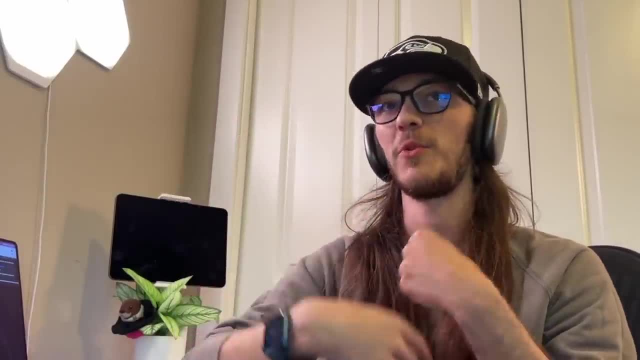 You know, can we teach you how to take ownership? Can we teach you how to, you know, be responsible for what you work in, to be passionate? Those are things you can't teach people. Now, if we back up a little bit, 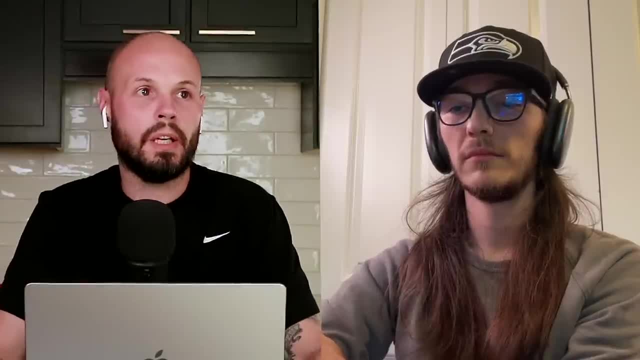 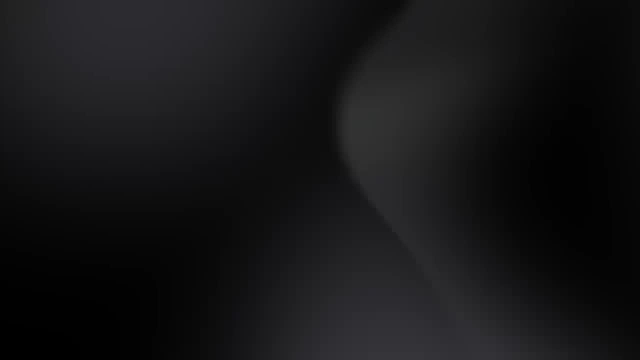 this thought just occurred to me. You're homeless, living in a car, sitting at McDonald's. iOS development is not a cheap game. to get into right You have to have a MacBook, You have to have an iPhone. How the hell did that happen? Connect those dots for me. 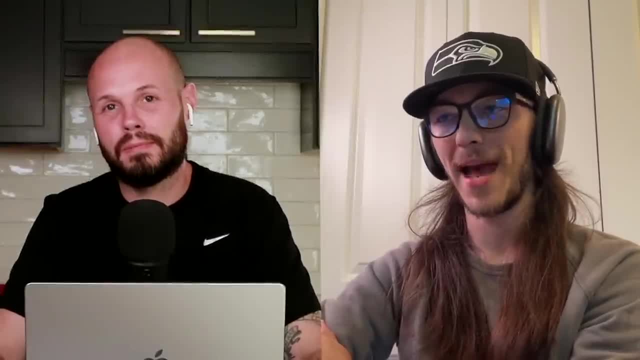 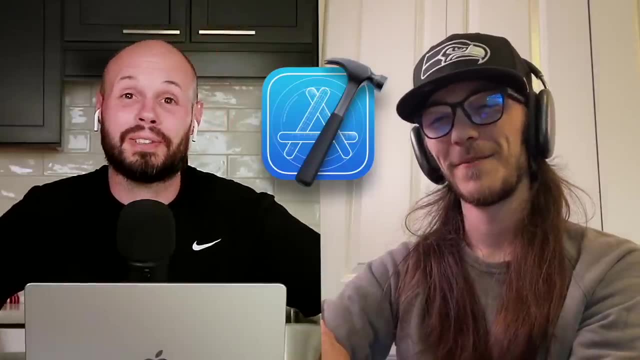 Definitely, definitely. So what was wild is I had an old like 2010 MacBook That I got from a friend. you know I used it for a little bit and it would not run Xcode for nothing. I can't imagine how frustrating that would be running Xcode on that whole machine. 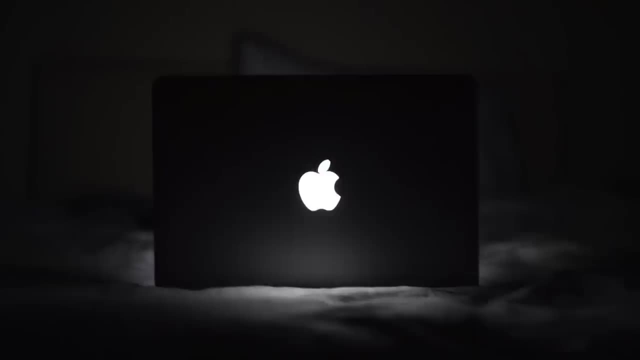 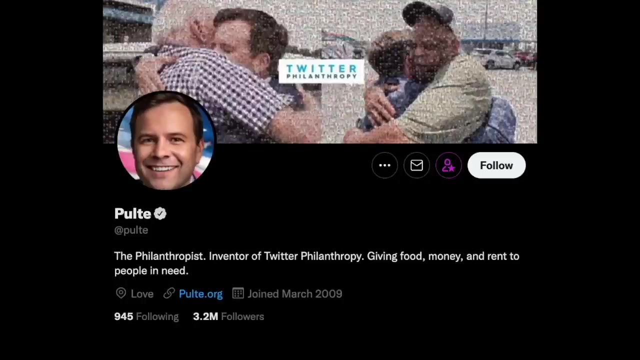 You're just thinking about it. Oh man, and it had the light up logo and everything. So, you know, I'm like sitting in McDonald's with it just feeling cool, Like I thought the light up logo was still new and modern. and I found this guy on Twitter named Bill Pult and he's like a multimillionaire and he's a philanthropist. 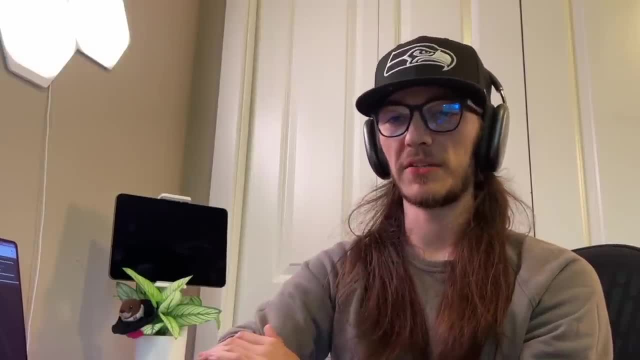 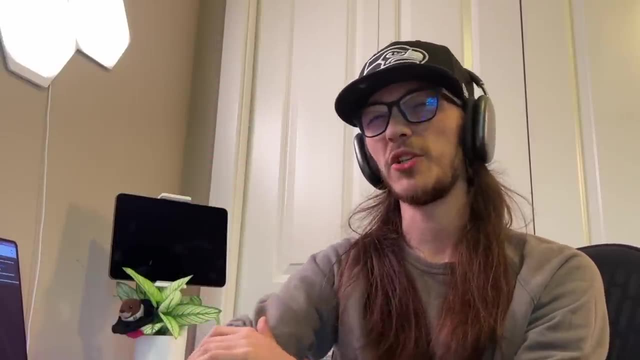 He gives away money on Twitter to people in need. I posted on one of his things or tweeted on it, you know, and I said I need a new pair of shoes and I need to get a MacBook for school and like, I gave him like a screenshot of my application. 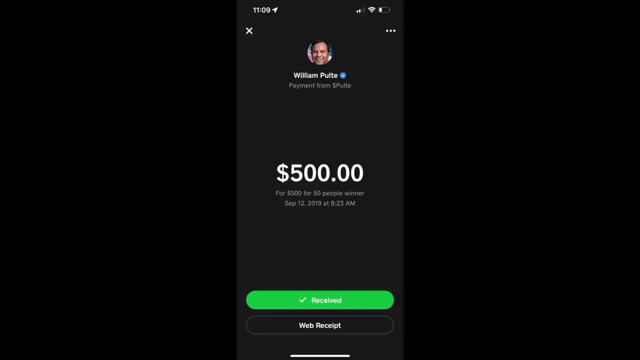 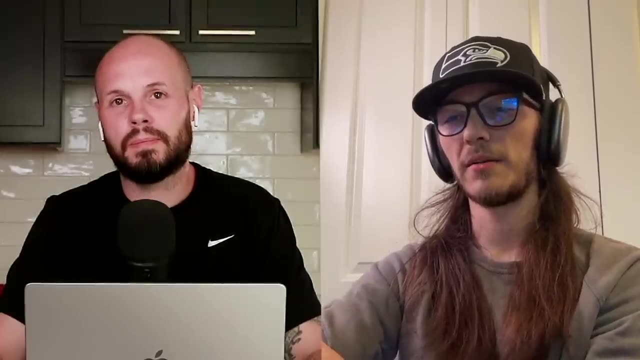 The next day I woke up and I had $500 in my cash app. I was able to take that money with my tax return, and then I took the old laptop to a pawn shop and I was able to get myself like a 2019 MacBook Air. 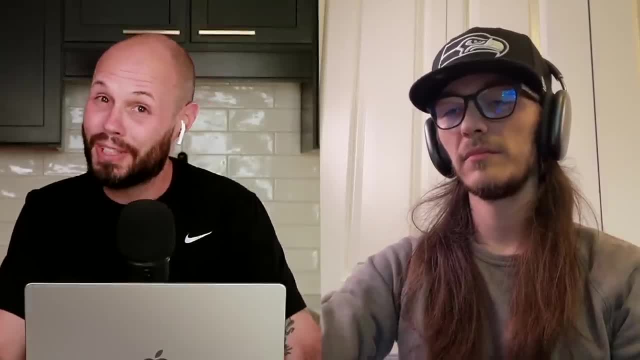 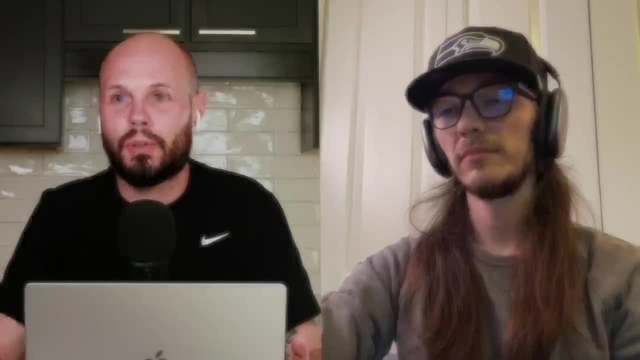 Now you're off and running 2019 MacBook Air- Still not the greatest development machine, but better than what you had. You also talked about getting these interviews with standing out, but you also said you didn't get any of the jobs. So how did you actually get your very first job? 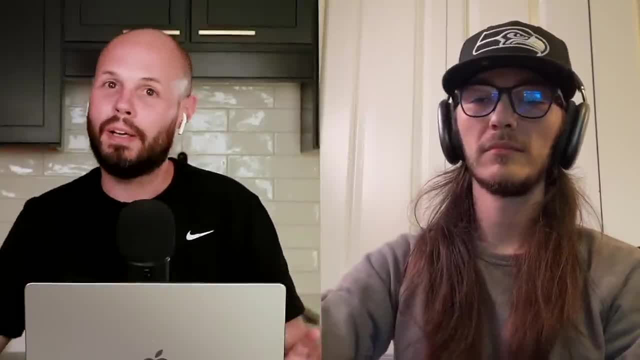 Because what I led with at the very beginning of the show was this: you know, mid six-figure job. That's where you're at currently, but there was a job before that. So how did you, how did you get that Through Twitter again? 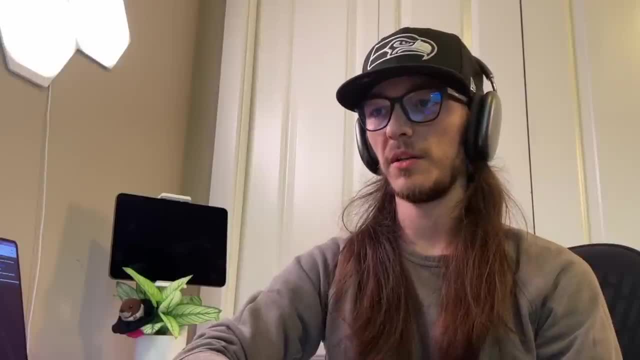 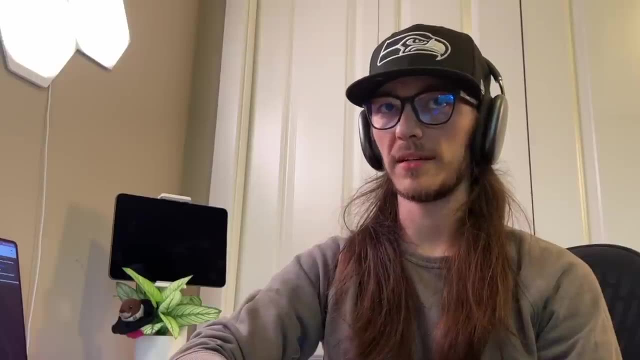 I was using Twitter to utilize, like the networking and, just you know, being a part of the community, and I ended up finding the- I think it was Cyril- and another person that did a Twitter iOS hackathon, and I had a friend named Nadeem and Nadeem- 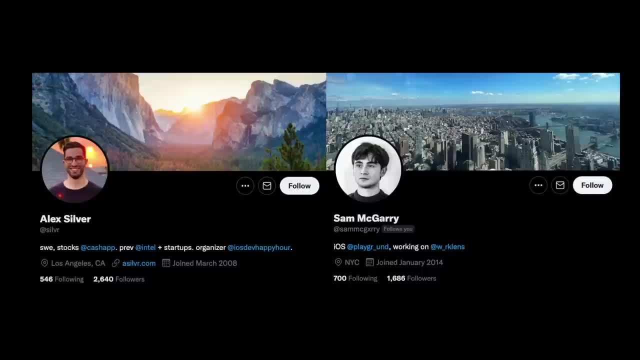 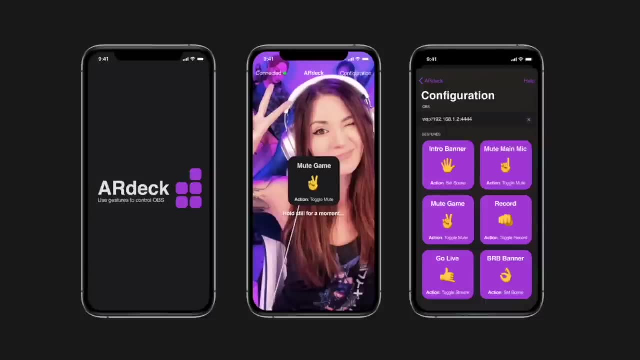 and I ended up joining up with Alex Silver and Sam McGarry and we did the iOS hackathon and we had a application called AR Deck. It was really fun. We built in 24 hours and Nadeem is like the most amazing developer. 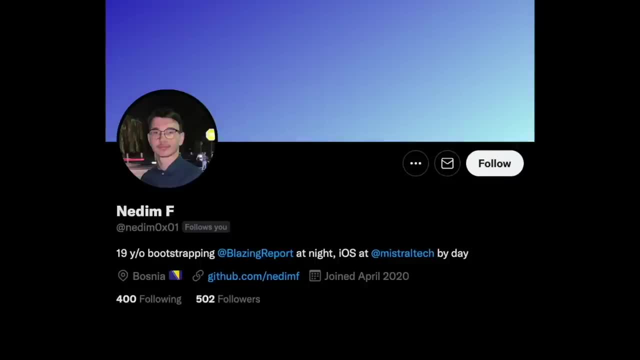 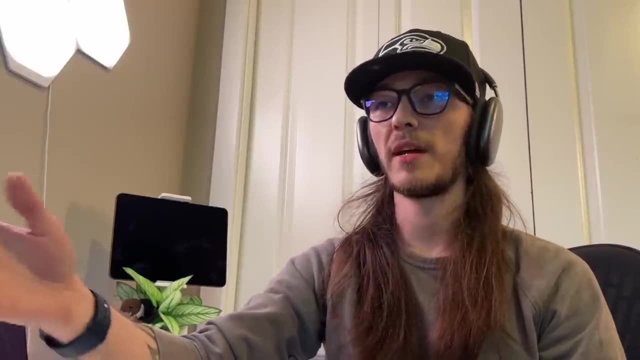 He's the most, he's the smartest developer I've ever met for his age, truly So. we built this application in 24 hours and somehow won, and I was just as surprised as all of those were. There was really great competition going on in there. 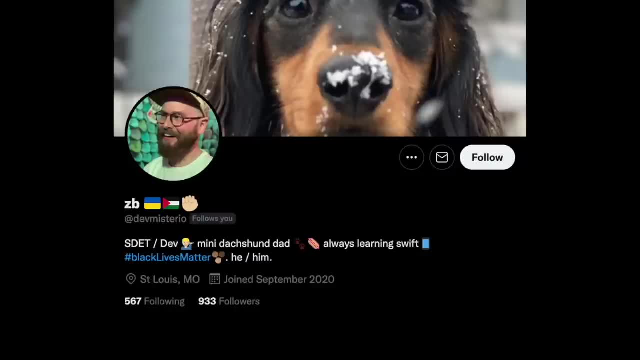 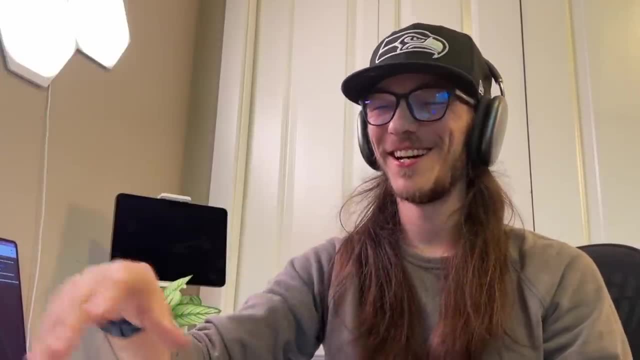 and all that networking and all the new followers I got led me to Zach Becker who, to this day, you know, I can't, I couldn't give back to that man, you know, more than I could ever could, because Zach noticed me and told me, you know, he just 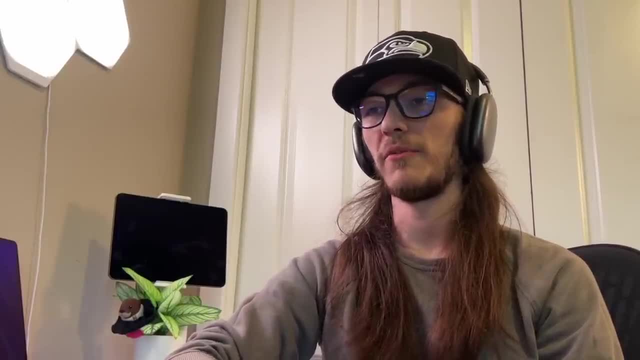 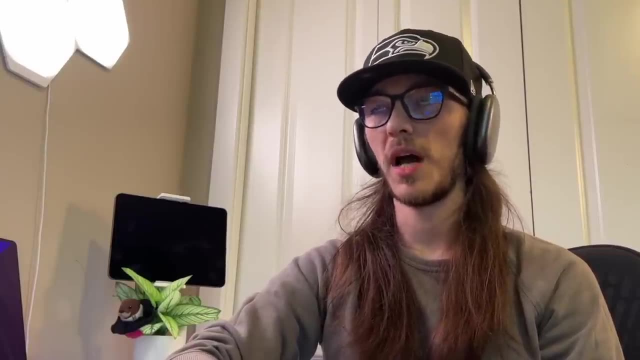 started chatting with me and everything and asked me about my developer life and, like what I've done, and I explained my life to him, my story, and he, kind of you know, told me that he was trying to pay it forward and felt, like you, I could do the work really well and he gave me a recommendation. 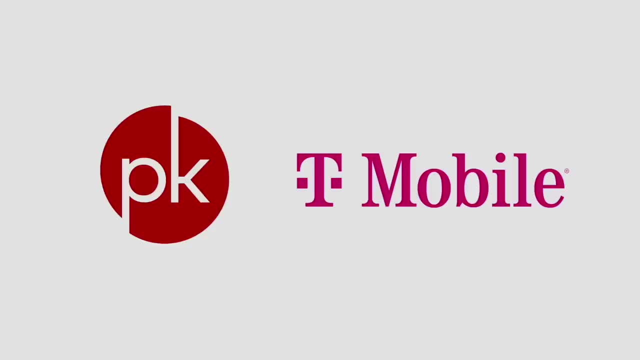 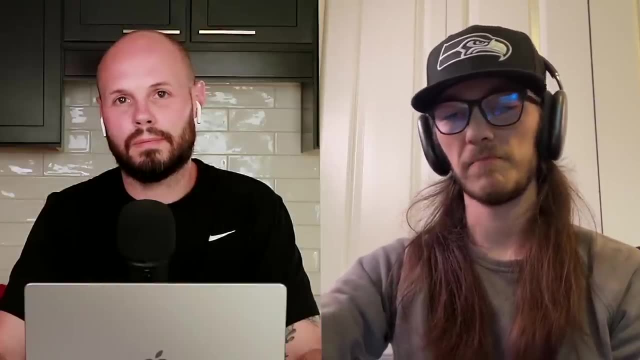 to apply for PK Global, which is one of the contractors for T-Mobile. so I went off with the races again I applied and, shockingly enough, they called me back and I got the job. So you mentioned that this was a contracting company for T-Mobile. so I guess when I hear contracting, I 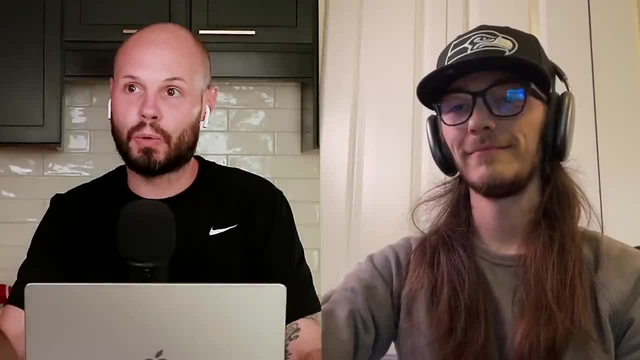 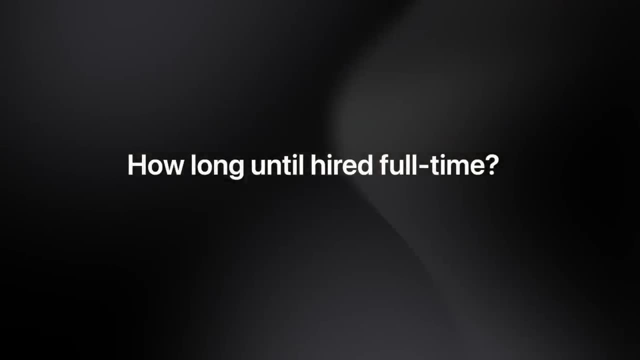 think, building a bunch of random apps for a developer agency, but it sounds like you were working at T-Mobile, just not as a full-time employee, as a contractor. so how long did you do that? because, spoiler alert, you are a full-time employee at T-Mobile right now. how long did that? 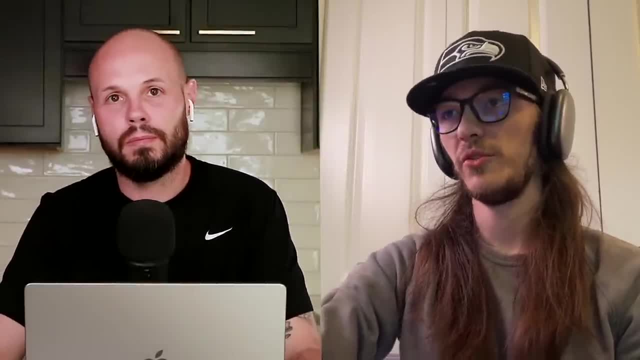 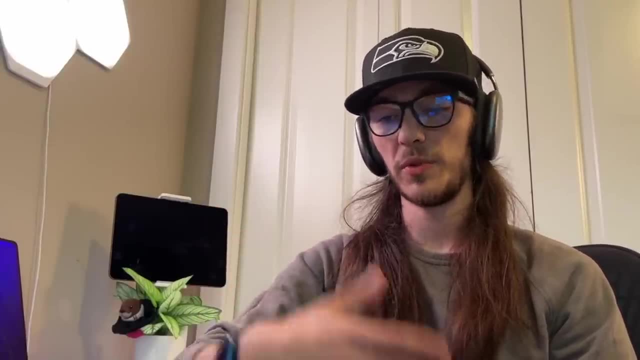 take and what was the process of getting hired full-time? In contracting you do kind of get thrown on random teams and everything and I was lucky enough to be thrown on the retail frontline experience. so I got to genuinely work with the and I still work with the application that we have across 8,000 plus T-Mobile stores. it's the front-facing. 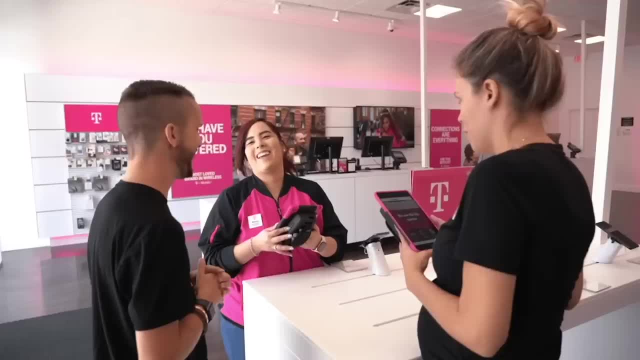 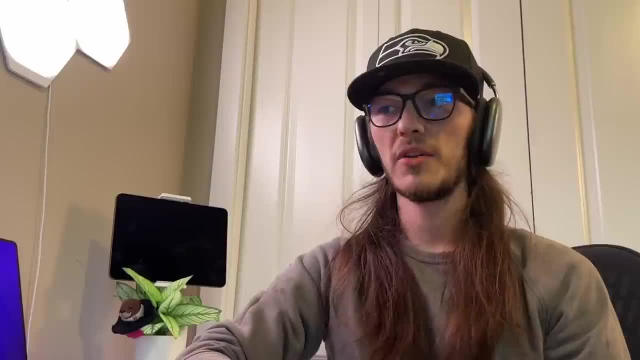 application that's used on the iPads across every single store, what the employees themselves use to actually sell your phone, purchase your phones, trade your phones and upgrade your phones. so I was able and lucky enough to be on a team that's important, you know, like I know, there's a lot of 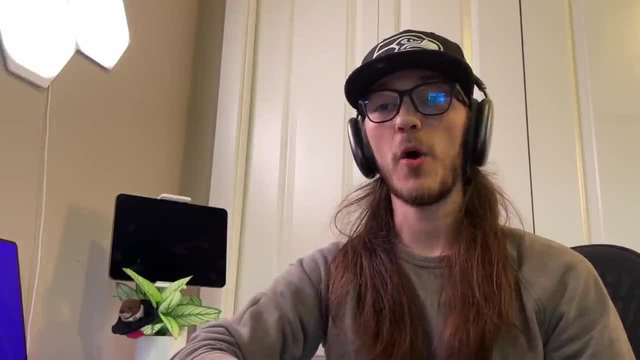 microservices and everything. so I had a lot of opportunity to really take ownership of my work. you know, like I know, there's a lot of microservices and everything, so I had a lot of opportunity to really take ownership of my work. we had, you know, I was doing automation work at first and we didn't 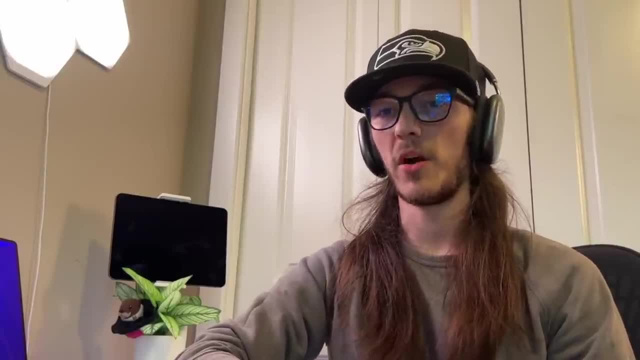 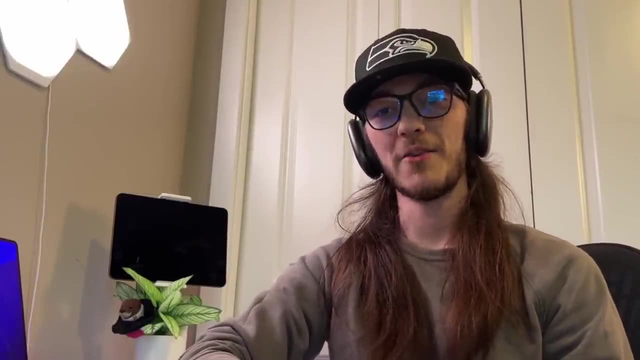 have an automation team that was really big. we didn't have anybody that was really leading automation at all, and you know I was. I guess this comes a little bit with naivety and also with, just, you know, excitement. I don't know if you know I was five years in the development in a company. this 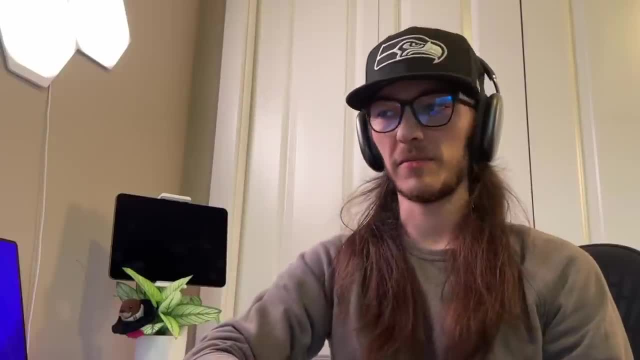 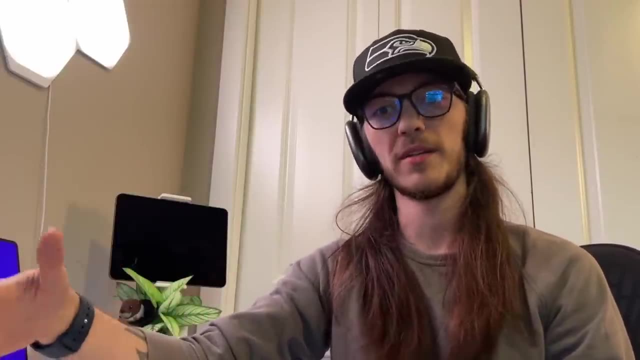 big, I probably wouldn't have done this again, but I just jumped up at the idea of: well, hey, you know I could, you know we can do this and this, and you know this is important to me and I want this to be done because you know, without this getting done, this won't get done. and just taking ownership of 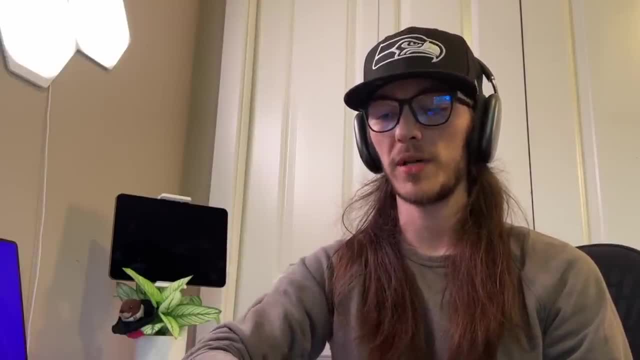 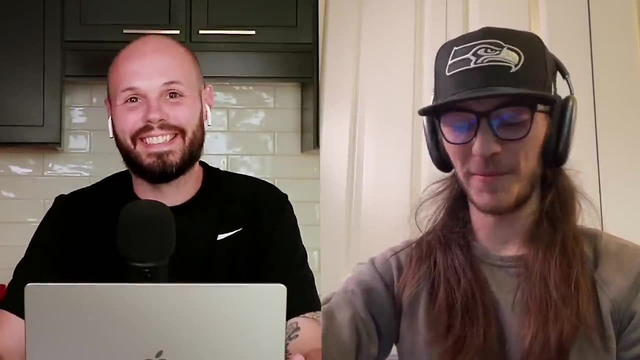 things and you know I was doing automation work at first and we didn't have an automation team. about seven to eight months I got a request and it was asked if I wanted to go full-time and I accepted. I didn't even think about it, actually jumped on it. yeah, yep, I jumped on it. 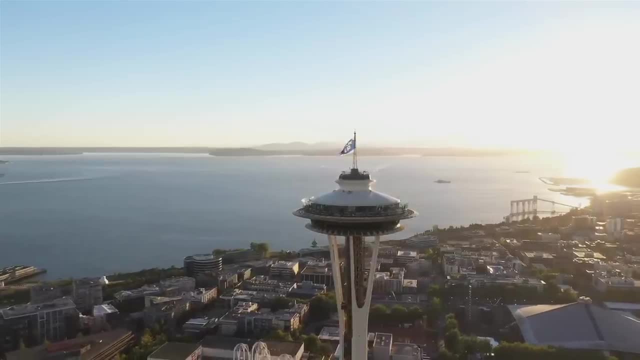 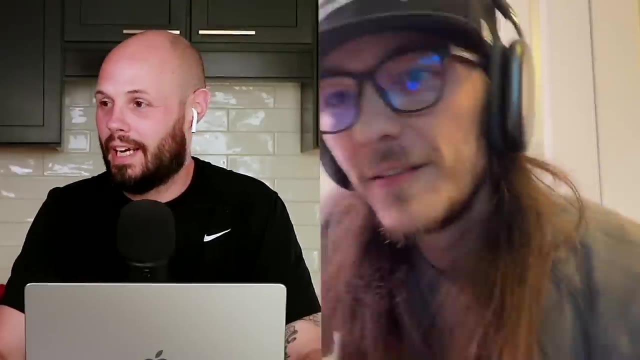 so quick. and next I woke up a month later and I'm living in Seattle, across the country, and definitely has changed my whole life, that's for sure. I'm really thankful for you, I'm thankful for everything. I appreciate that and that's. I mean that's awesome. here you are, that's where 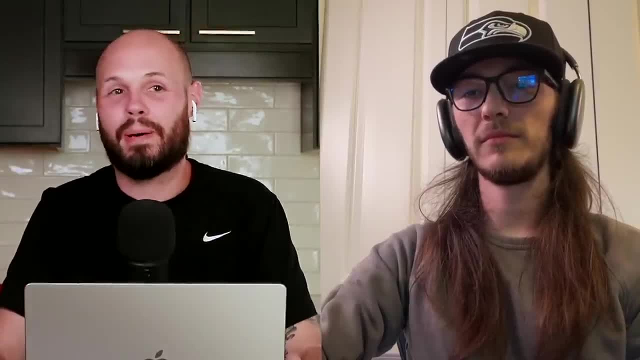 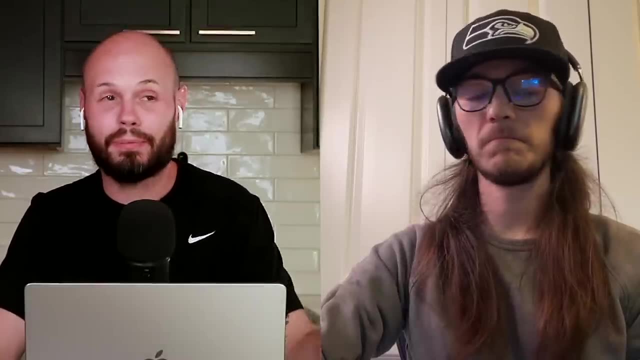 you are right now. that's that's kind of the whole story getting up to present and I just want to recap. like you know- you mentioned it earlier- not only do you not have like a college degree- I think you said, you don't even have a high school degree or a GED, right, and you're from. 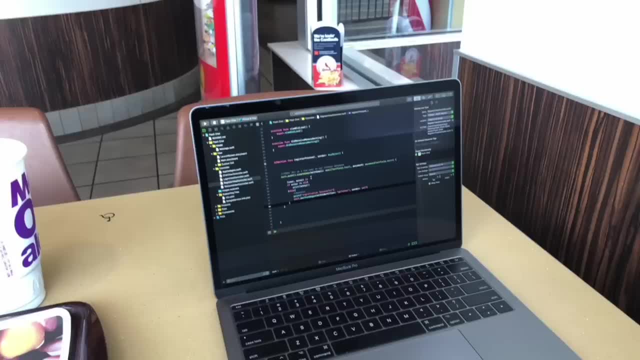 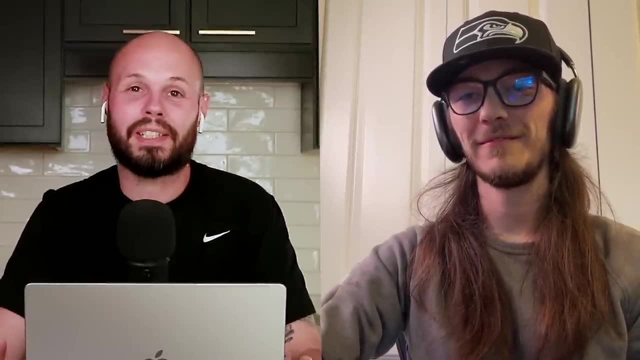 homeless in a McDonald's parking lot stealing wi-fi. so now here you are, full-time software developer, mid six figures, like that's. that's an amazing story and, like I said, I'm so happy to share this. I can't wait to see like the comments and the reaction, like I think it's awesome. so 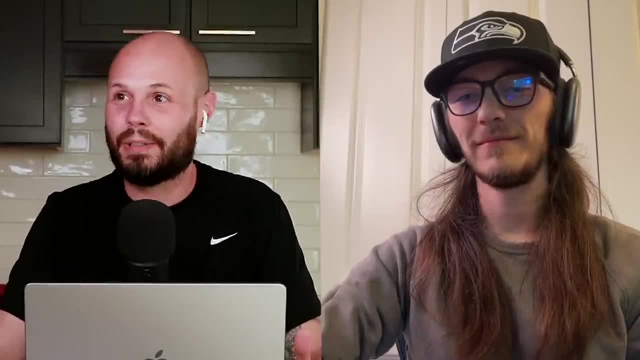 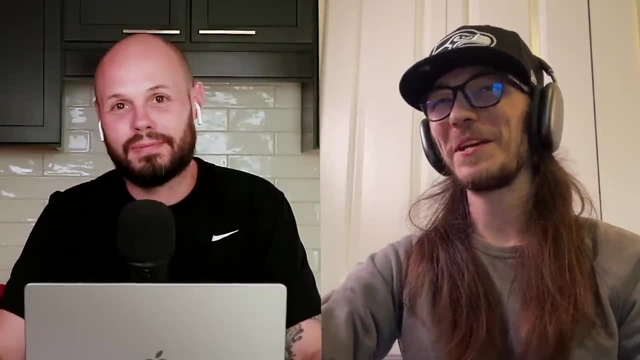 not to discount like how far you've come in this awesome story, but I gotta ask, like what's next? what? what are the next two, three, four or five years have in store for Ezra? like where do you want to go? yeah, definitely, I think that I'm going to focus on stability. 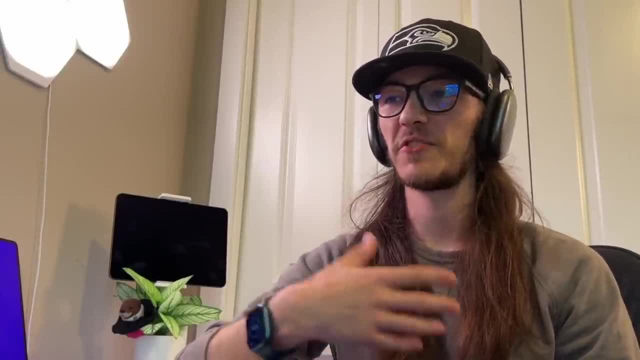 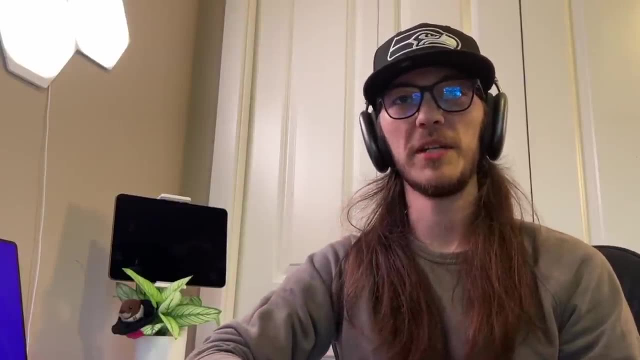 and financial growth and in terms of my career and everything, augmented reality is right around the corner, you know, and that's where I like to focus. I enjoy fiddling with all the bleeding edge technologies and a lot of my obsession right now is in LIDAR. so, hopefully, once we start getting 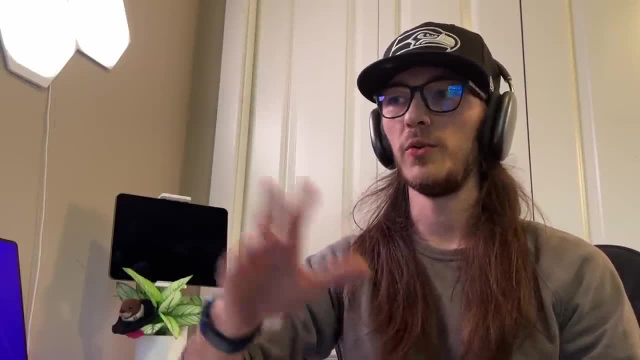 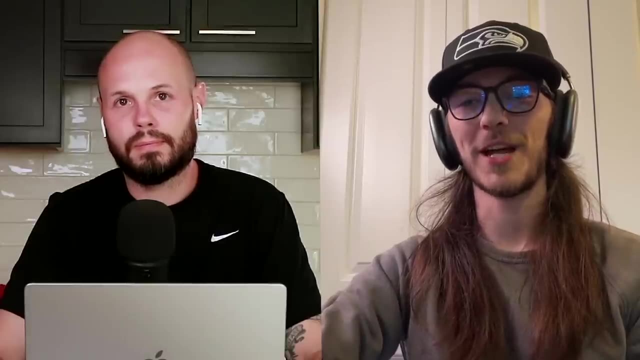 like the hardware to catch up with the software. there'll be a whole new wave of something for me to enjoy, maybe ride that wave as well. so we'll see. but it's probably going to be something to do with augmented reality. I've kind of been watching from the sidelines, a little bit like. 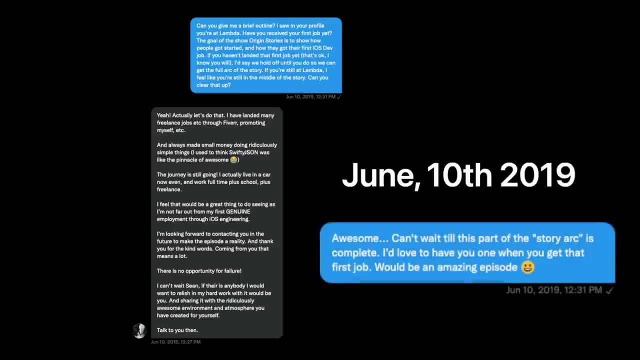 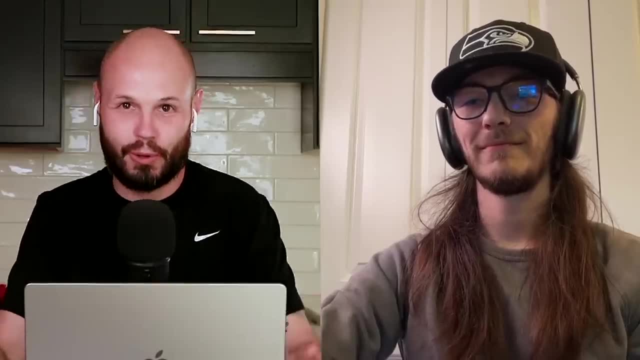 I said at the beginning, you reached out probably two years ago. you know telling me where you're at with your story and kind of been. you know keeping keeping tabs a little bit here and there and it's just awesome to see kind of like it all come to fruition with where you are now again making well into the six. 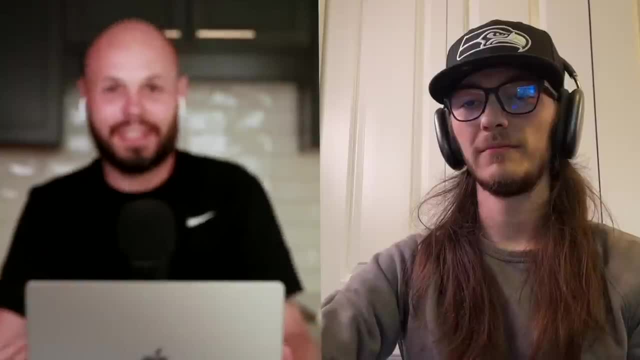 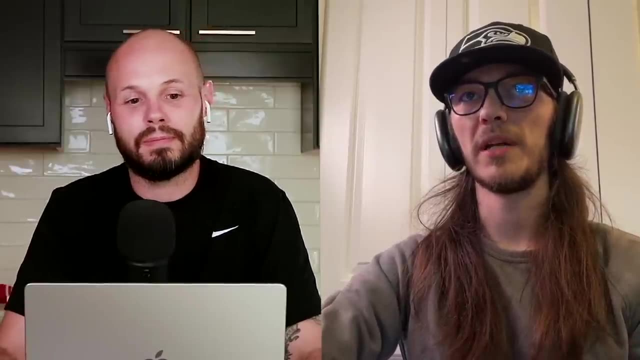 figures. so I know you're excited to share your story, but I'm just as excited, like I said, I can't wait for people to hear this and I think it's going to be inspiring to so many people. you know, that's all I really hope for. I mean, if it wasn't for your videos and getting inspired myself, I 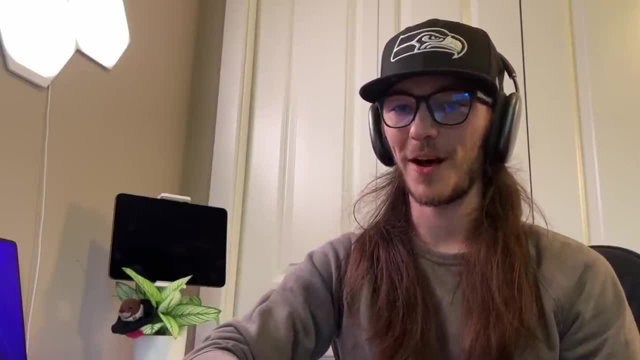 wouldn't have had nothing. you know, and I feel like everything starts in your mind because it obviously does, and if you just have a little bit of time to do that, I think it's going to be interesting to have that a little bit of drive and focus and the want to have better and stop. 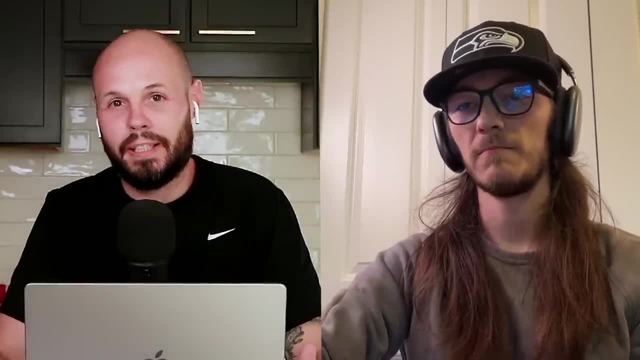 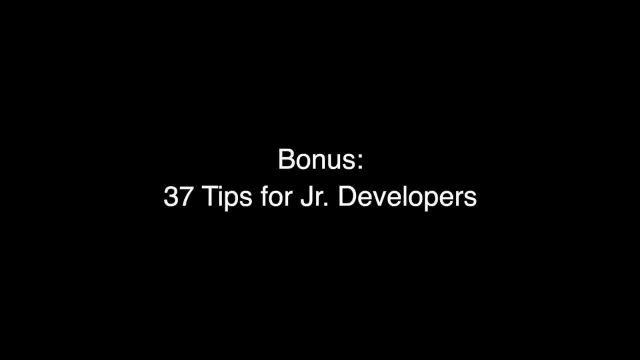 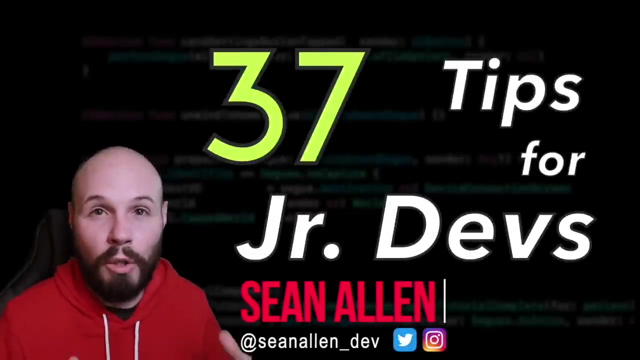 discounting your future. you're going to get places. just focus. it's great way to end it well. I appreciate you coming on, Ezra, and we'll see you all in the next video. yeah, definitely appreciate you. what's going on, everybody? today we're rattling off 37 tips or pieces of advice for junior software. 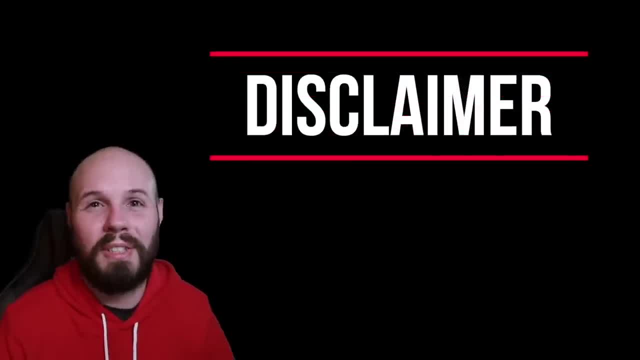 engineers, and whenever you put together a list like this, of course there's going to be some exceptions. so if you have some thoughts about my tips, leave a comment below and I'll see you in the next video. bye, bye, let's have a discussion, throw 10 minutes on the clock and get right into this. I got a list right. 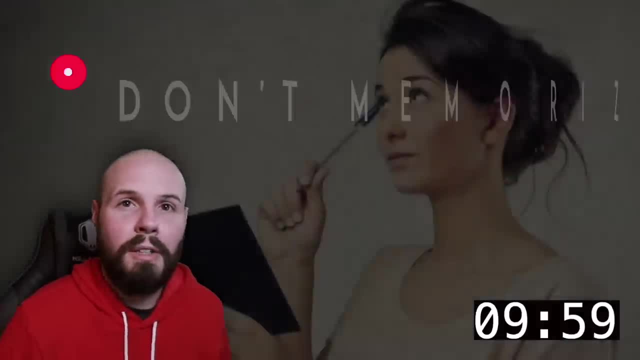 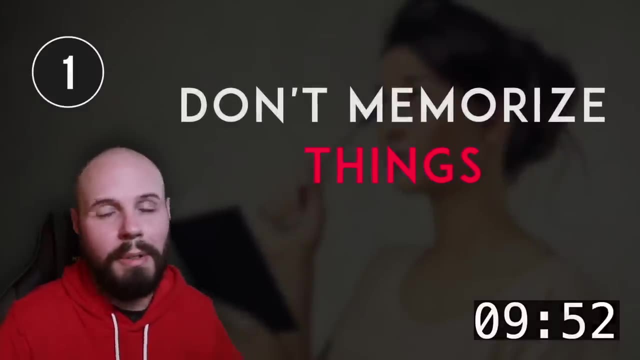 in front of me and these are really in no particular order. but number one: don't worry about memorizing things, right. I think a lot of people think that they have to know how to build everything off the top of their head. they just go there and type, type, type, no, even the most senior. 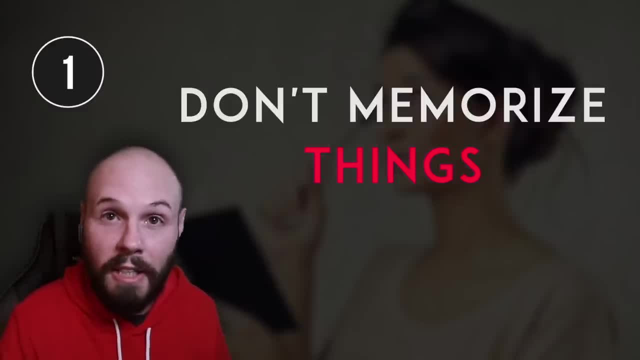 developers google the most basic stuff all the time. the key here. you got to know where to find it, whether that's previous projects or you know where to go in the documentation. that's the name of the game. know where to find it. don't worry about memorizing number two. you got to learn how. 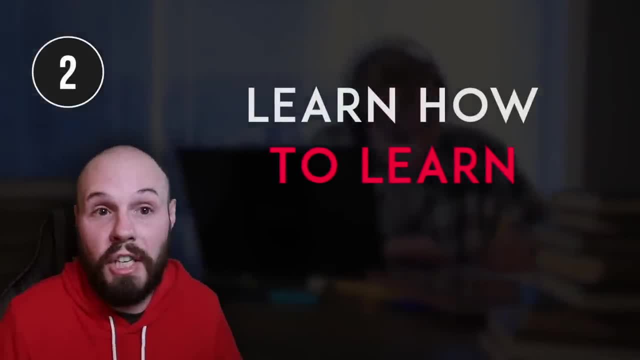 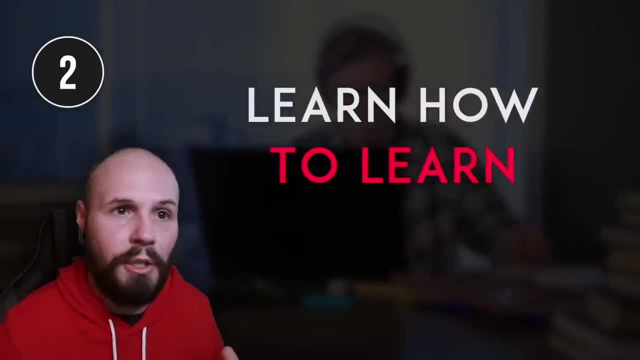 to learn right. this industry is constantly evolving. technology is constantly changing. the one thing that will be constant is that you're going to have to learn new stuff all the time in this career, so learn how you learn- whether you're an audio learner, you like to read books you like. 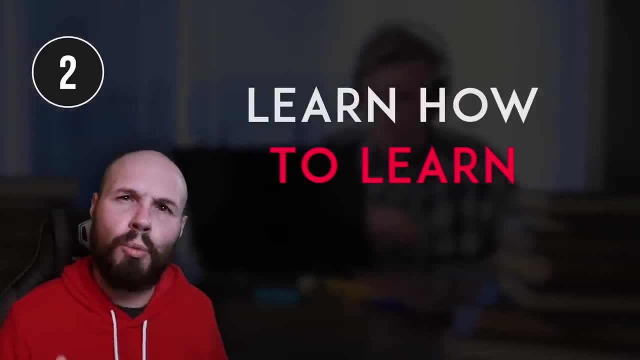 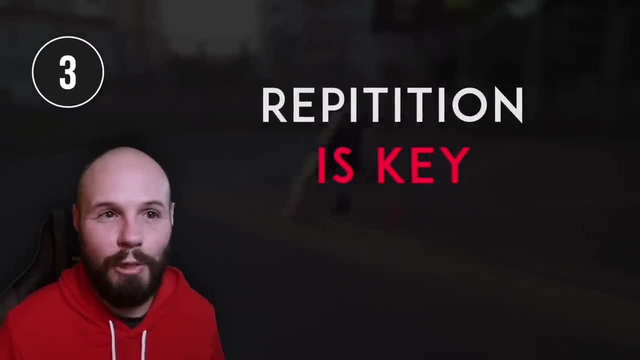 to watch videos, figure out the best way you learn things and get really good at that, because you're never going to stop learning in this career. and number three: sticking with the learning topic. repetition is key, right? you don't just learn one thing in programming and then you know it, right? 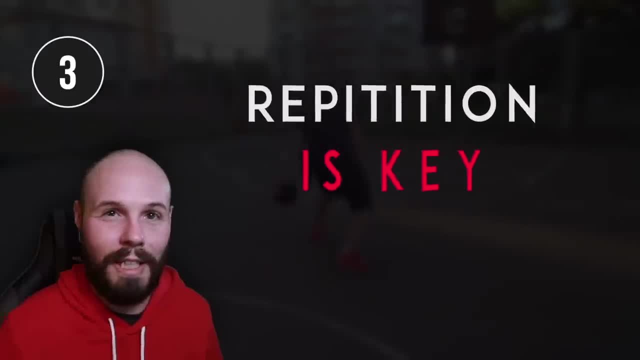 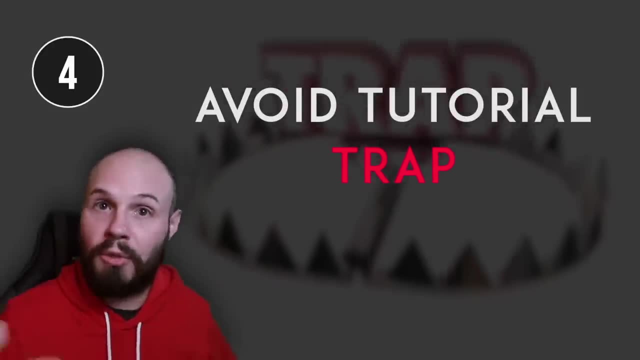 you know it by doing it over and over, and, over and over again. repetition is the key. number four: don't fall into the tutorial trap. i think a lot of people, when they're just learning, do this tutorial, do that tutorial. they just do endless tutorials. your learning will really take a leap when you start building your own projects. when there's no. 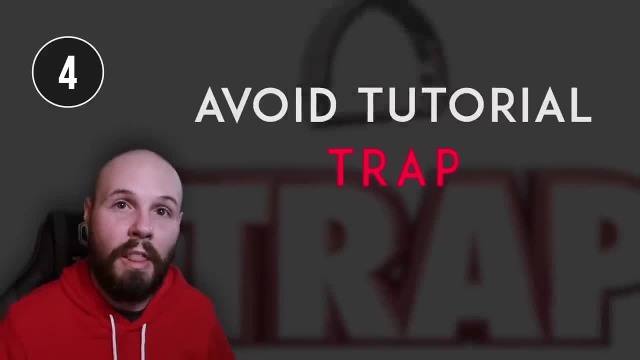 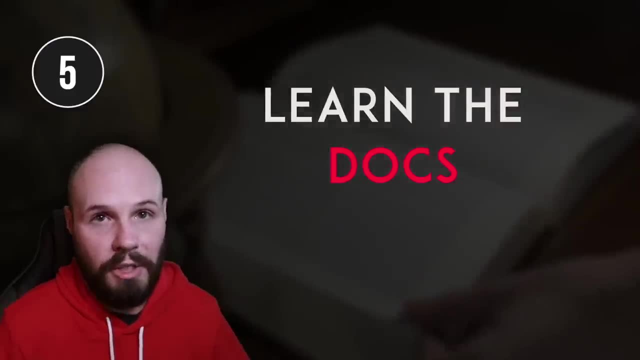 cookie cutter recipe for you to follow. you got to figure it out on your own. that's when you're going to take the leap as a developer number five, and this will help you get out of that tutorial trap is learn how to read the documentation for your language. i understand not every language's. 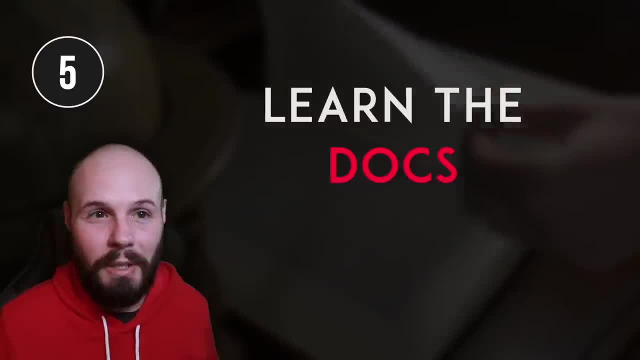 documentation is created equal. some are great, some are not so great, but that's what you got to work with. and knowing how to read the documentation, how to use the documentation as a resource. again, that gets you out of the tutorial trap. you're not relying on other people's tutorials. you can dive. 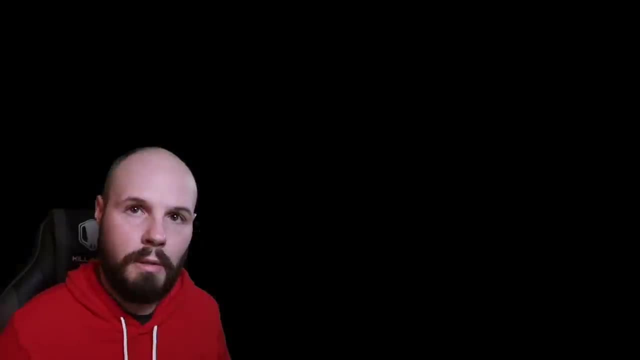 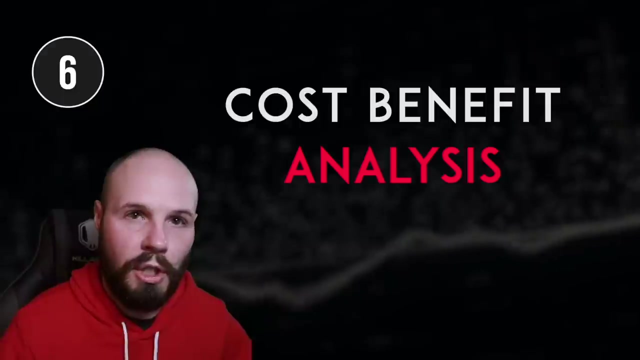 into the documentation and figure it out for yourself. that is a vital skill. number six: this goes along the lines of once you're actually working on a project- is learn to understand the cost benefit analysis of your work. a good way to think about that is: each feature has like a 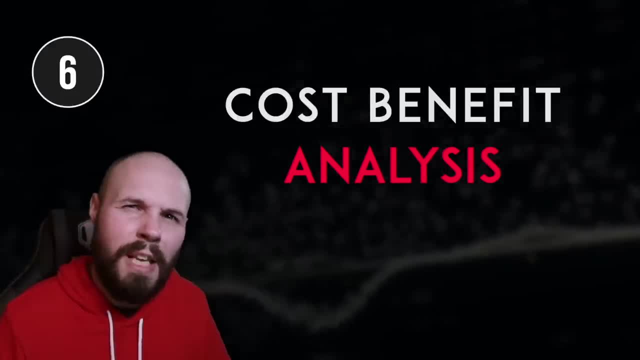 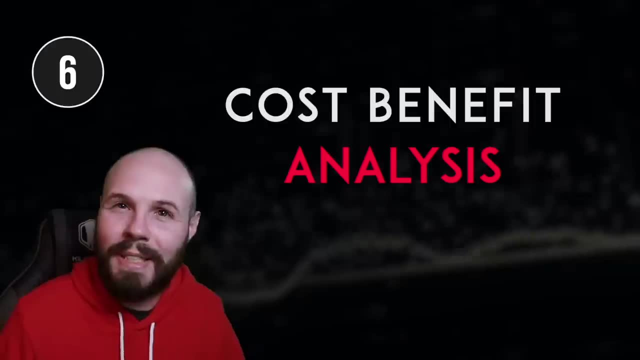 spectrum of complexity. right, you may have an idea for a feature. there may be a super simple, easy to implement version of that. it may not be as robust as it is, but it's going to help you learn how to do it as you want it. but again, you got to manage how much time it's going to take you to build it. 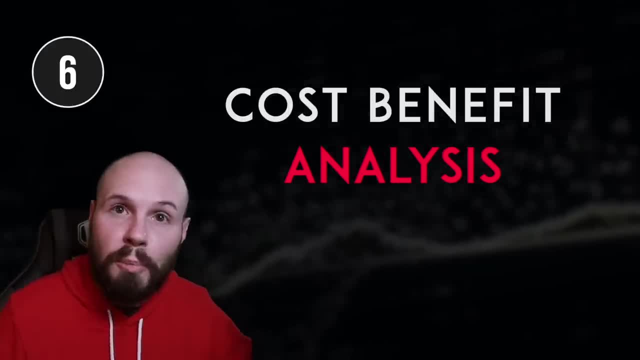 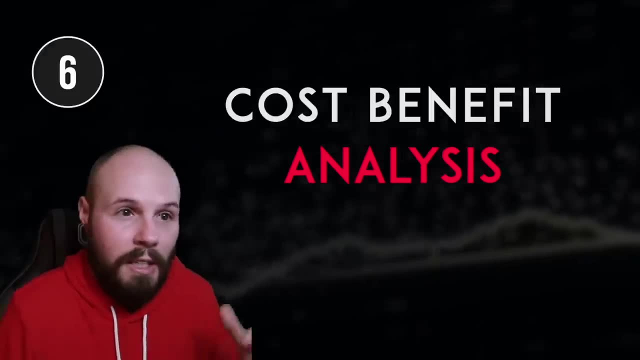 versus the benefits you're going to get. so, along that spectrum of super simple basic version to really complex robust version, there's a whole spectrum of versions in the middle. so learning to balance that cost benefit analysis of the time you're putting into it is key when you're building. 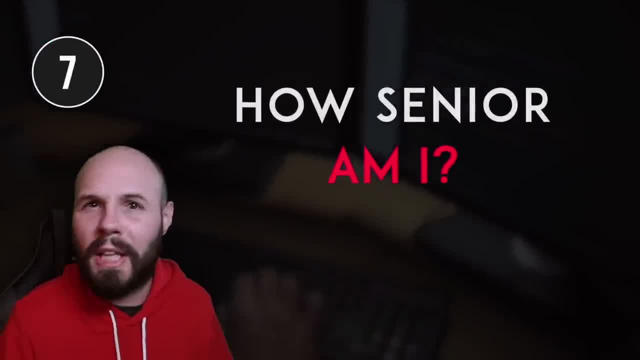 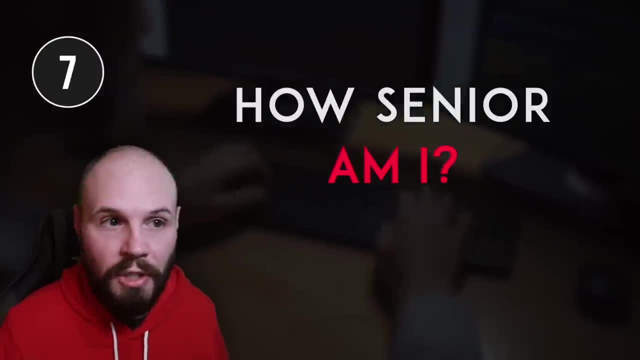 products. number seven. let's talk about the. am i a junior developer, mid-level developer, senior developer? when can i call myself what? i think that's an irrelevant question. don't even worry about that. you could ask 10 different developers. you're probably going to get 10 different developers. 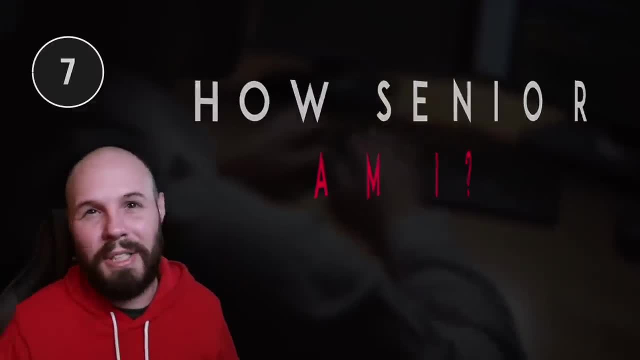 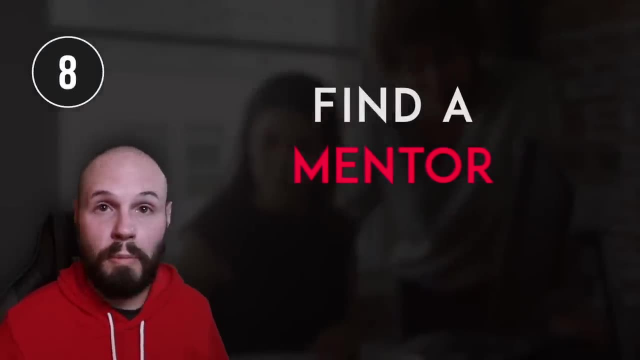 it's very abstract, very vague. stop wasting your time thinking about that number. eight: find a mentor, if you can. whether you have somebody in person that you met at a meetup or, you know, maybe build a relationship with somebody on twitter. finding a mentor early on can make or break. 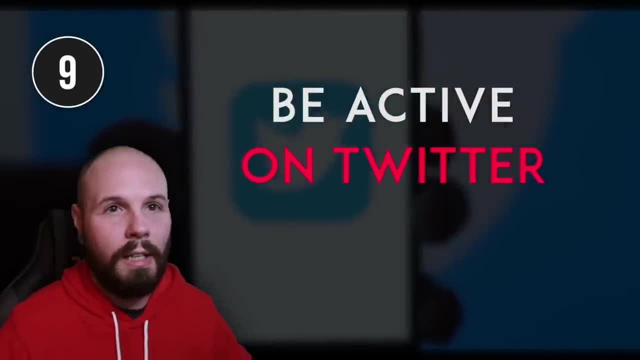 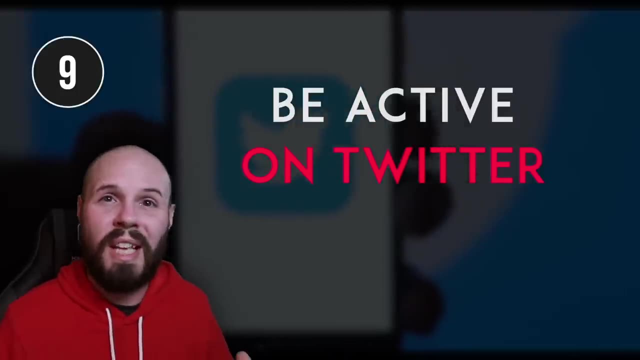 your career and along those lines. number nine join twitter. uh, developers hang out on twitter. it's where they talk and communicate. it's an amazing place to network, especially if you don't live in a development hub, but use this as to build relationships over time, like i consider twitter. 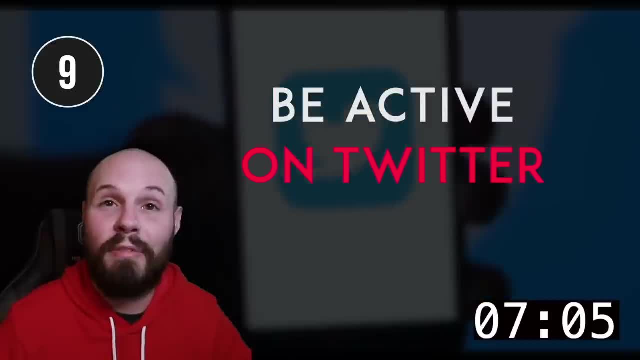 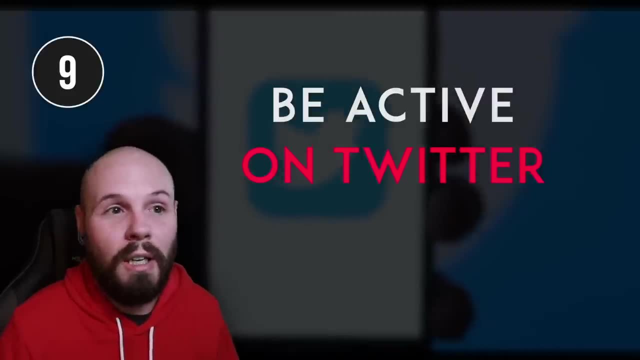 probably the most powerful tool in my development world and i think it's going to help you build a developer career. just the people i've met, the networking i've done- i've gotten job interviews for dming people i know on twitter. it's just, it's amazing. build your twitter, uh, join the community. 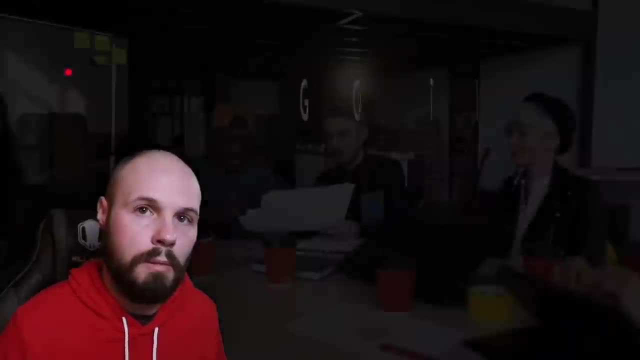 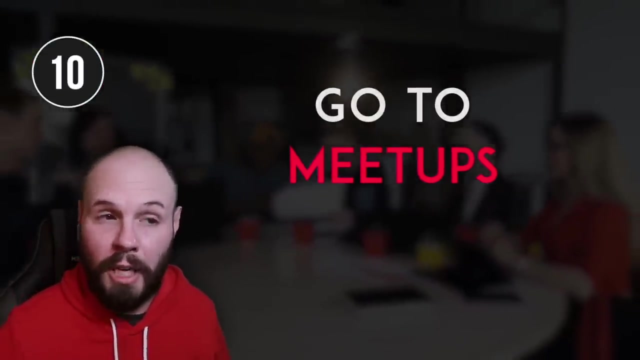 be active, be known. it's one of the most important things in my opinion. moving on to number 10, go to meetups if you can. i understand- uh, you have to be in a bigger city to probably do this, um, and twitter is a good backup if you're not, but if you can go to in-person meetups, so valuable your. 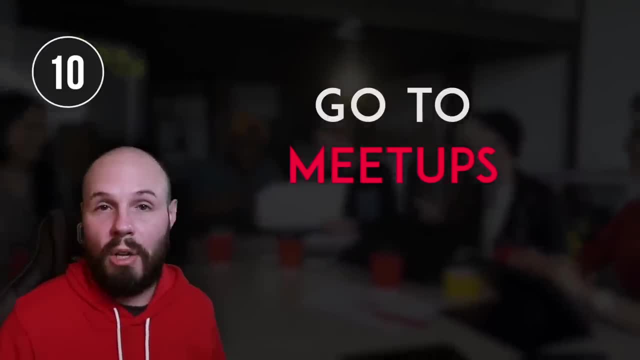 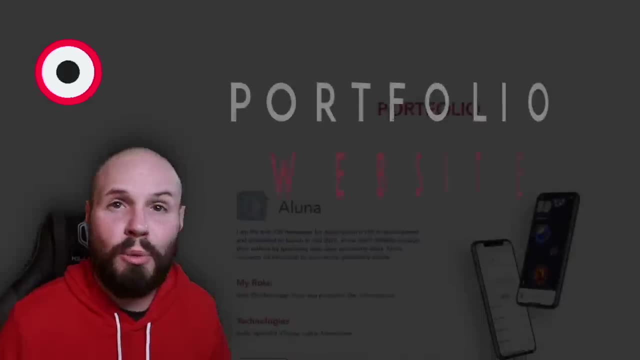 network is your net worth. i mean, so many career opportunities happen based on: oh, i met so-and-so. like it's just, it's real, it happens. go to meetups if you can. number 12 might be the most important on this list and i genuinely believe in this, but if you're a junior developer, you have to create a. 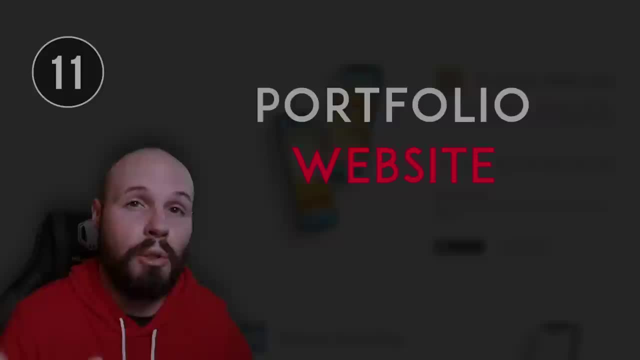 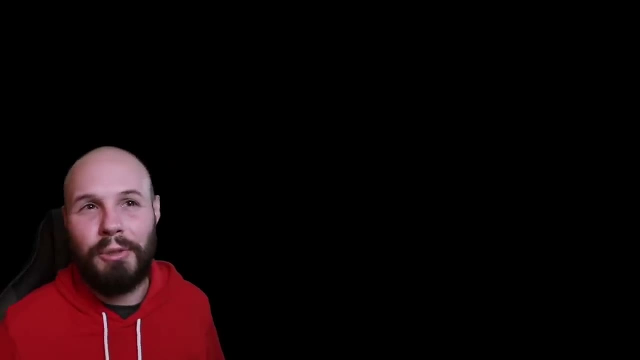 very visual uh portfolio website. you gotta showcase your work and apparently i don't know how to count. that was tip number 11, not number 12, off by one errors, am i right? anyway, tip number 12 is to create smaller portfolio projects. i believe you need to create a lot of smaller projects that can. 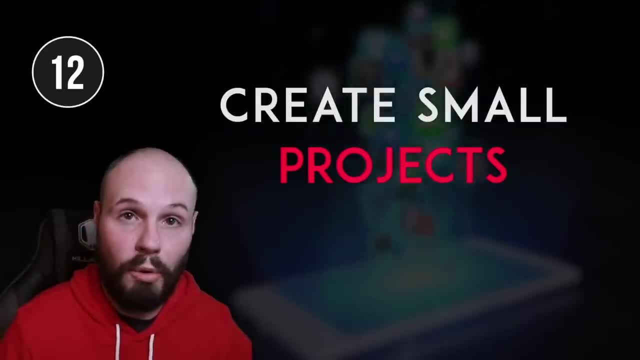 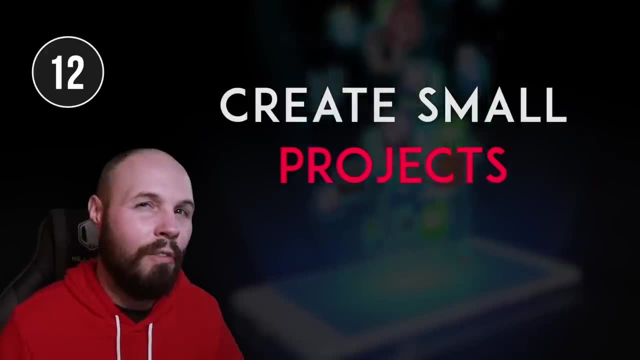 demonstrate a lot of different skills and showcase that on your portfolio. don't get me wrong: there's a lot to do in shipping a full product- like actually completing it, but at the same time, if you do that, you may only have one. i think it's also good to show many different examples of what 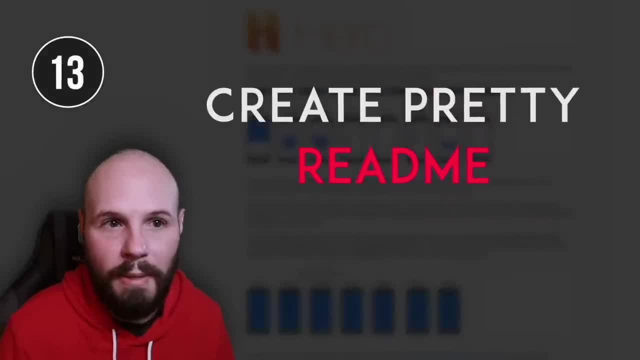 you can do. moving on to tip number 13, that is, your github repo readmes. make them visual, you know, put in pictures of the website or app you're working on. animated gifs are even better to show in action, but it's. it's pretty bad when you go to a github repo, the readme is empty, or if it's just a. 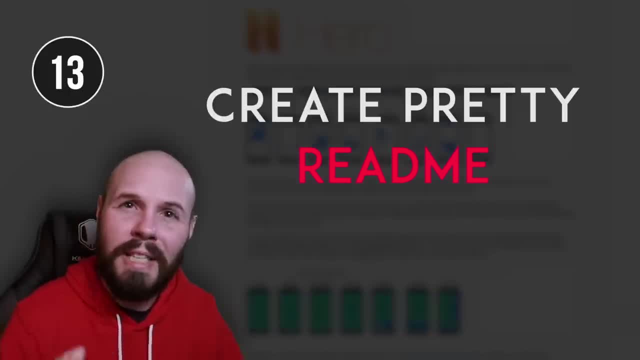 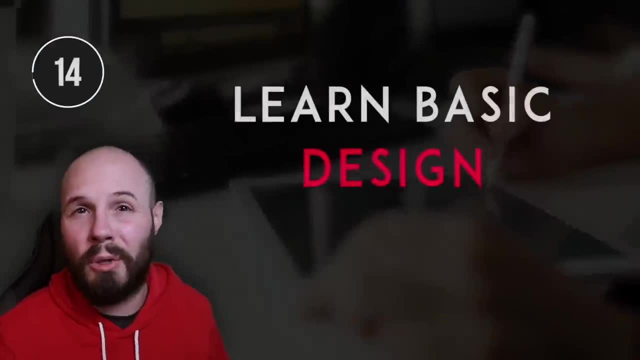 paragraph and then you got to dig in the code to figure out what it is. having nice looking pictures in the readme, awesome, do that. and number 14 is along those lines and just in general. but i think developers should have a basic level of design skills. i'm not saying you need to be a professional. 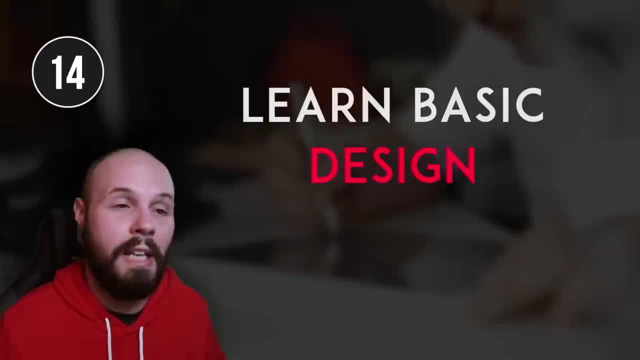 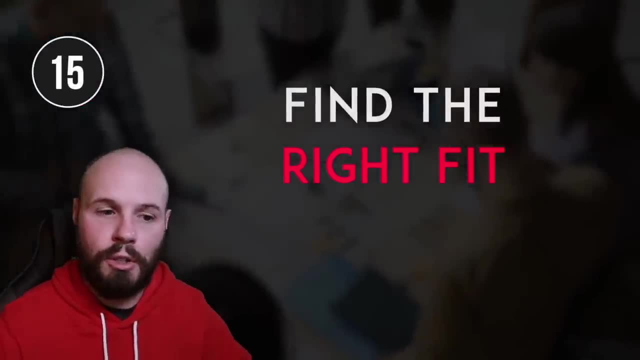 designer, but you should have some understanding of design. in my opinion. if you're making consumer products like apps or websites, all right, let's talk about some job stuff. number 15- and this goes out to those that are trying to get that first developer job, because this is hard, i get it, but 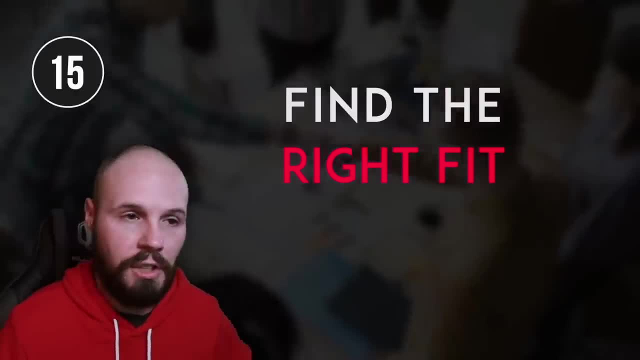 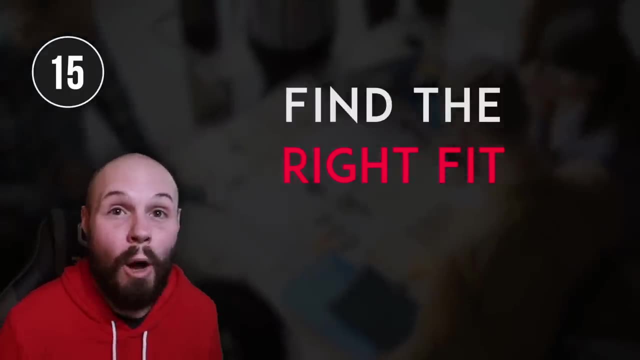 try to find the right fit, not the first offer for your first job- and i know like it's hard to get that first developer job. so the first offer you get is amazing. you're super pumped like hell. yeah, i'll take anything. i'm gonna ask you to fight that a little bit because your very first job. 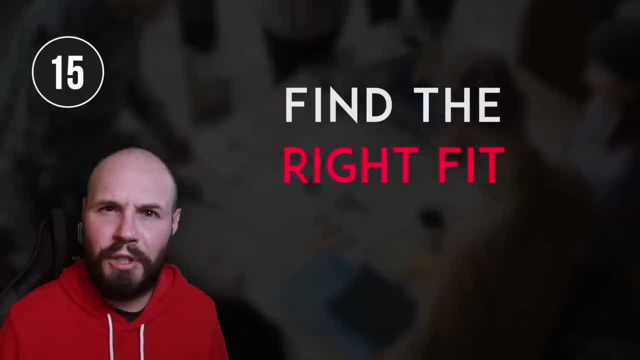 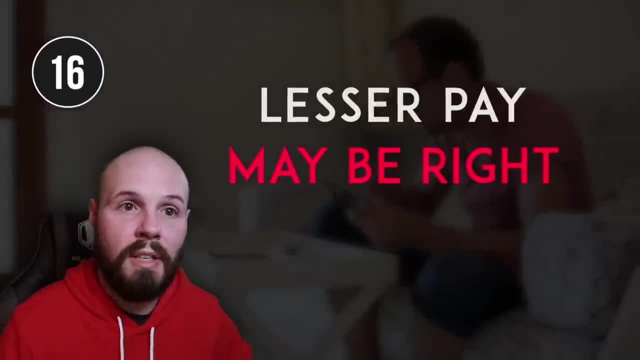 can either catapult you and launch you or hold you back, because you learn bad habits and it's not a good experience. it can really make a difference in the direction of your career. number 16 is along those lines. uh, and it's maybe a controversial one. i'm sure i'll get some push. 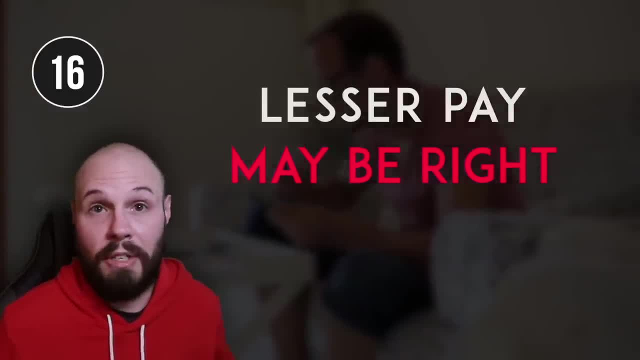 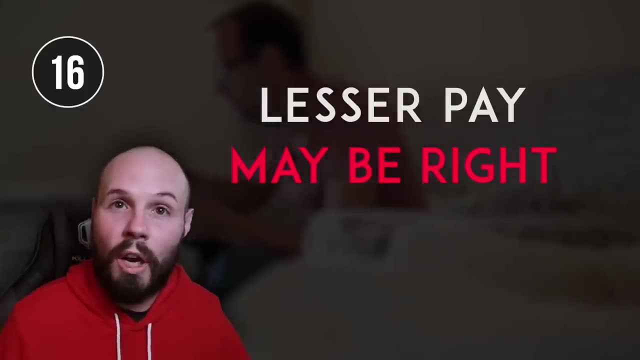 back in the comments. but take less money if you have to, if it's the right fit. uh, just using some american, maybe san francisco- numbers for you to figure out how to get that first developer job. say, maybe a job is 75 000 one offer, but it's an amazing fit- and another offers 90 000 a year. 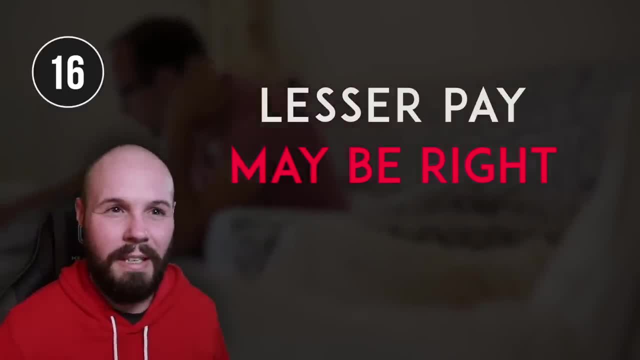 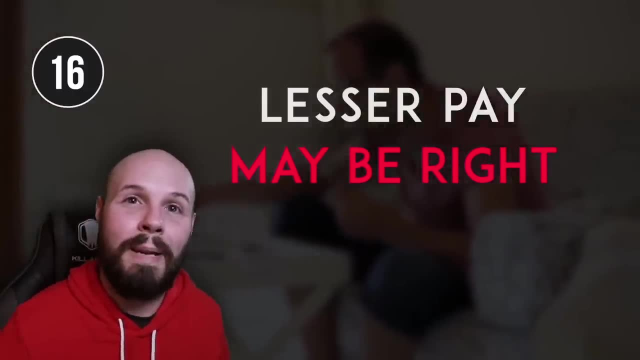 but it's kind of a crappy fit and doesn't look great like. yeah, you know, fifteen thousand dollars a year is a decent amount of money in difference, but i'm telling you it will compound over time to take the less money for the much better team, better product, better fit- that is going to outpace. 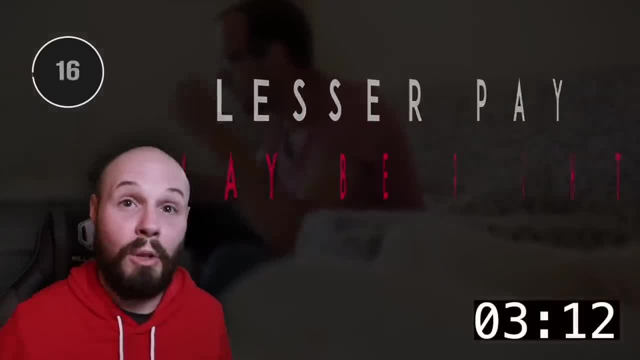 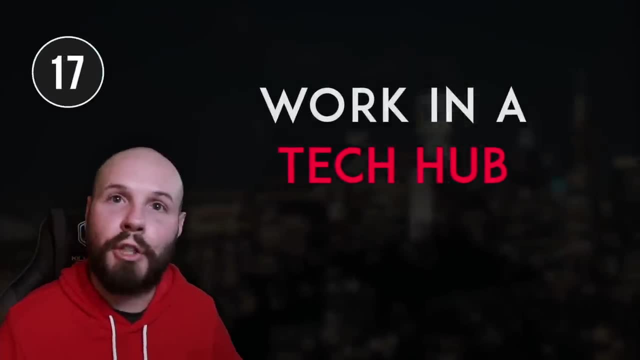 that extra 15 grand by a mile. uh, in the long run all right. number 17, and i may get some pushback for this as well. but i think you should spend an early chapter, and again a chapter of your career, in a major tech hub. you know the san francisco's, austin's, london, a big city with a lot of tech in. 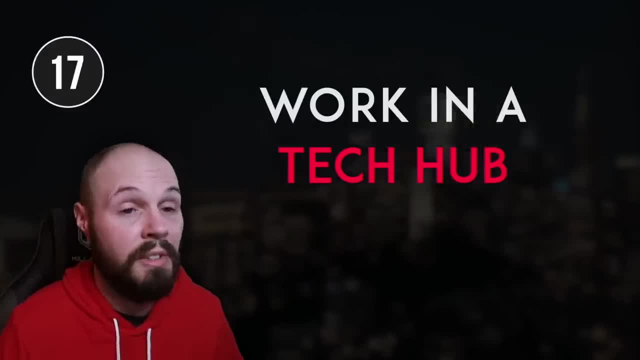 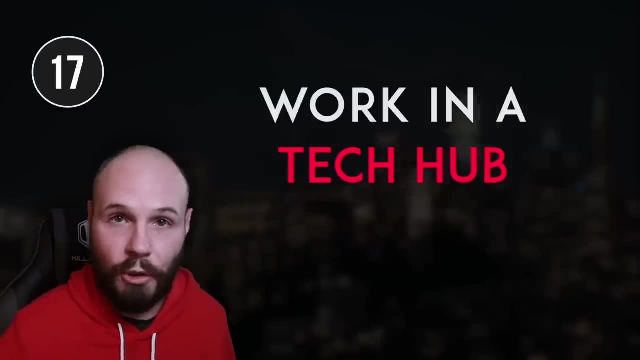 it and you know of course there's pros and cons with that. usually those are very expensive, uh, but the network you're going to get living in a tech hub is amazing and, again, can compound over the whole course of your career. so i understand people may not want to live in a large city like san. 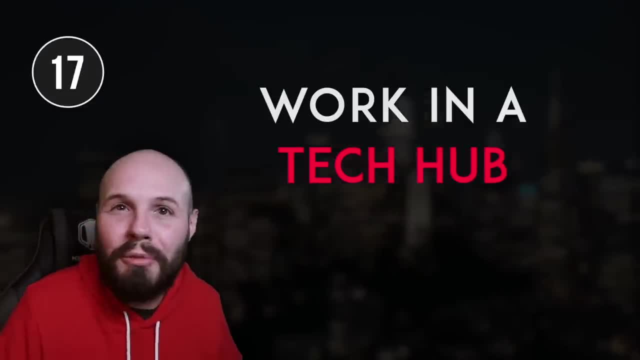 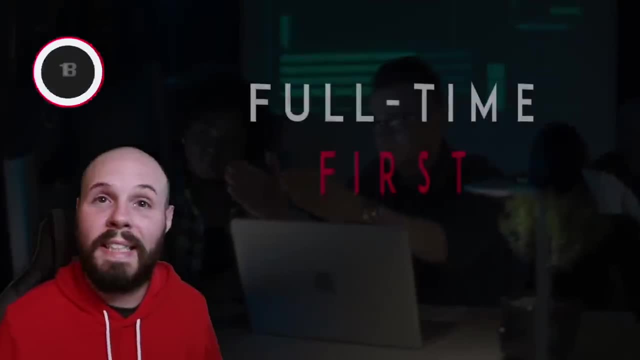 francisco because it's expensive, but just do two, three, four years there and then move on and, just like i said, the network you're going to get and take with you for the rest of your career, so worth it. number 18 is a contracting, freelancing kind of tip. i would do a full-time job first and start contracting and freelancing on the side as like a side hustle, to kind of feel it out, get used to it before jumping in full-time. i think a lot of people want to start their careers as full-time remote contractors, managing the project themselves. that is the dream. i understand why you'd want that. 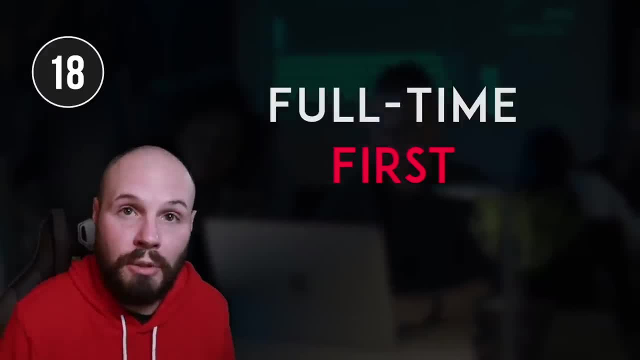 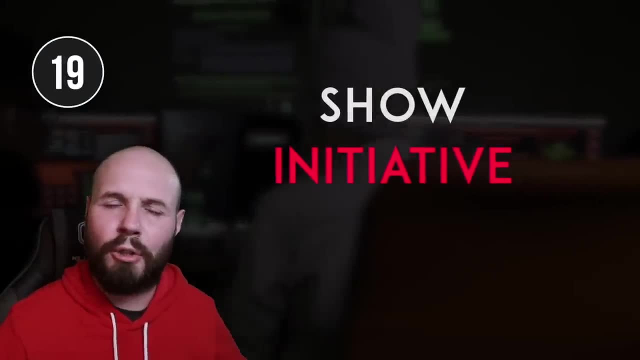 again for the long-term health of your career, i think it's very beneficial to start off at a do the contracting as a side hustle for a little bit and then switch. number 19 is just a general tip throughout your career and that is show initiative um, show that you care about the. 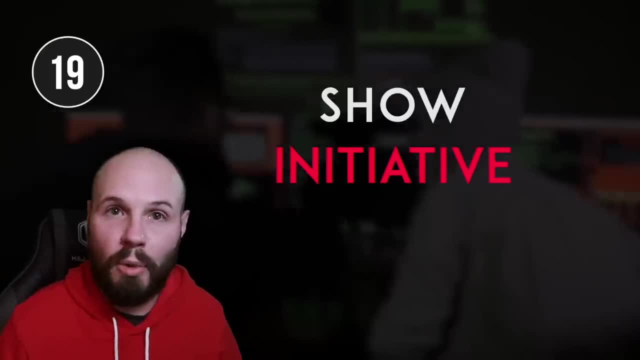 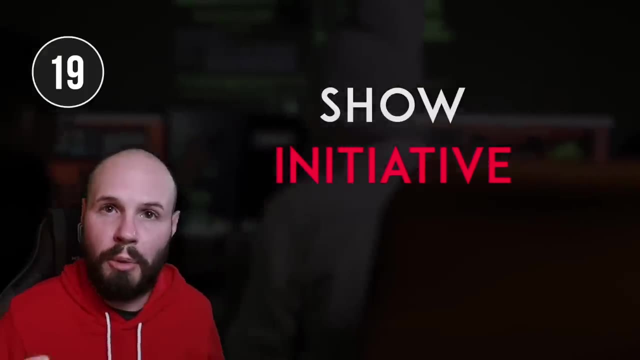 project. so if you're a junior developer on a project and you want to implement this one feature, go to your senior developer and say: hey, you know, i want to implement this feature. i think it'd be really great. i put a lot of thought into it. i think we could do it this way, this way, this way. 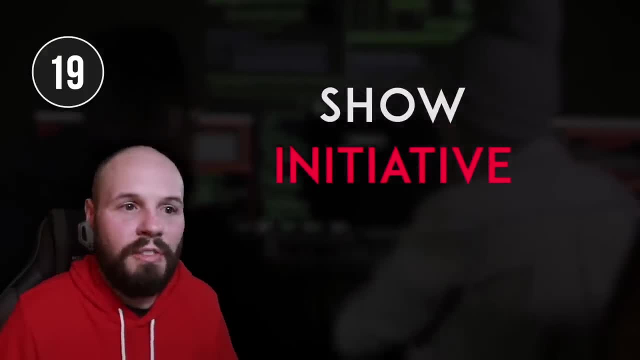 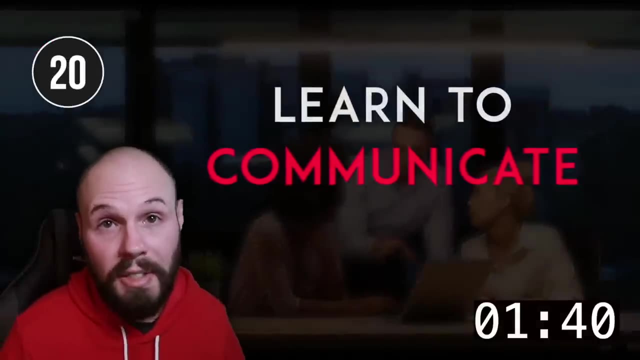 what do you think, even if they turn you down, just showing the initiative uh is going to be valuable. and just apply that to like all kinds of cases again throughout your whole career. number 20 is another crazy tip. i would do a full-time job as a side hustle for a little bit and then switch to. 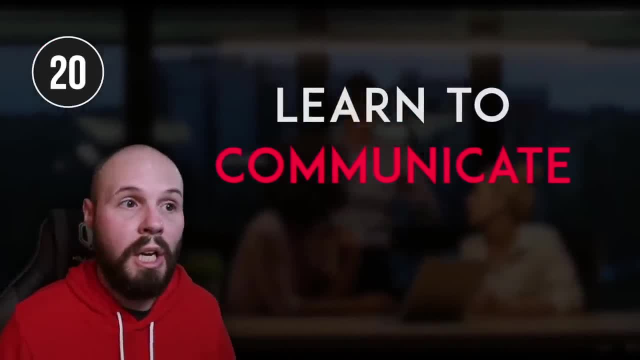 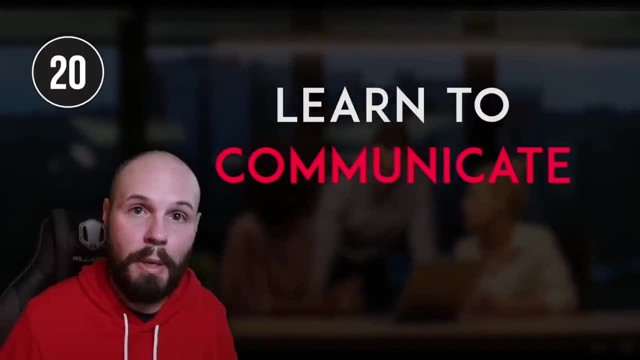 the important skill, and just in life, and that is learn to communicate better. if you can, as an engineer, break down these complex engineering problems and explain that to either project managers or maybe the ceo, if you're in a smaller startup, and making them understand like, why this? 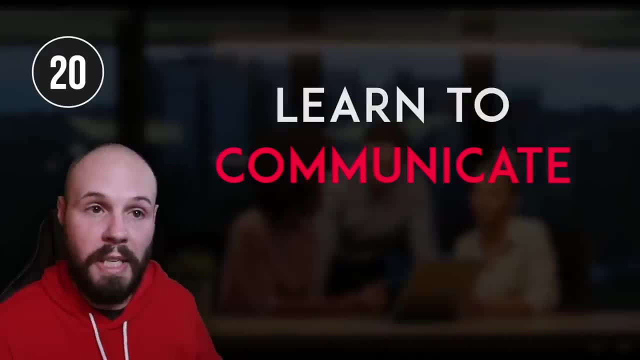 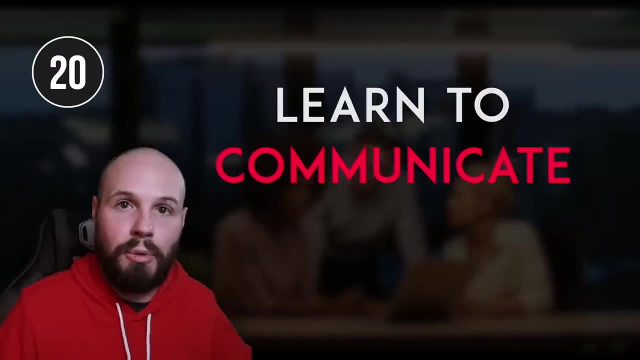 is taking so long, or the trade-offs between solution a and solution b. being able to explain that to engineers is one thing, that's a. you got to do that too. but being able to break it down into you know layman's terms for non-engineers and helping them understand again, that will make 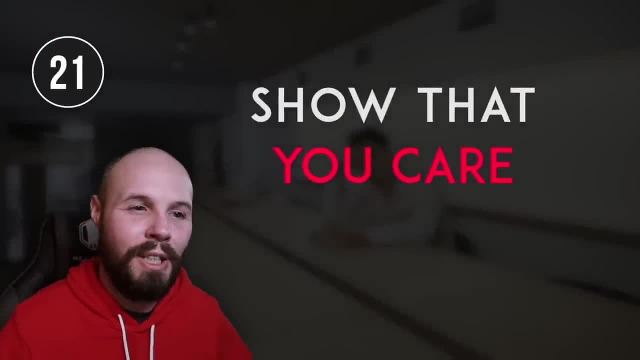 it so valuable to your company. number 21 again: when you're working on a team, just show that you care and this kind of goes along with the showing, the initiative. but we all know that person you work with or have worked with in the past that you can tell they're here for the nine to five. 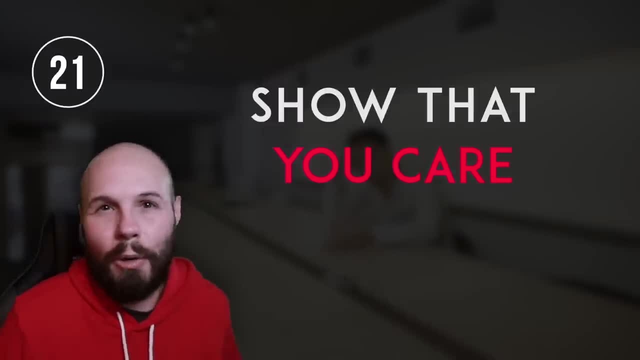 job. they hate being here. they're just here for the paycheck. they don't care about what's going on like you've worked with that person. hopefully you weren't that person. but don't be that person, uh, because again your reputation will follow you through your whole career. so if you are showing 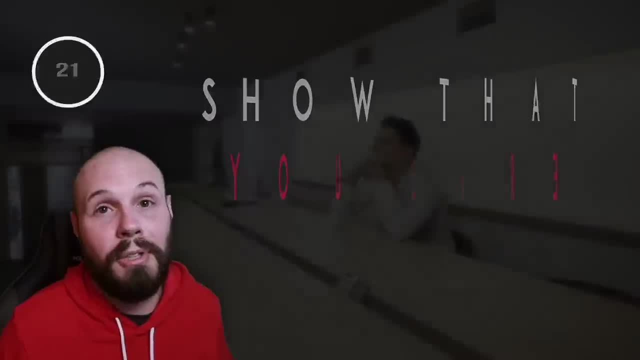 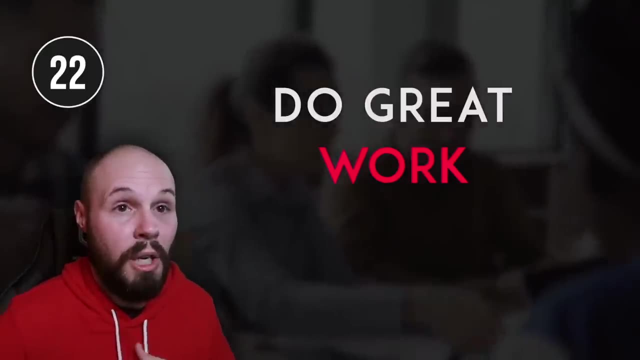 initiative, you show that you're passionate about your work. uh, that's going to go a long way and long way for your career and along those lines, number 22 impress. everywhere you go, like i just mentioned, your reputation will follow you, especially if you're in a tech hub like san. 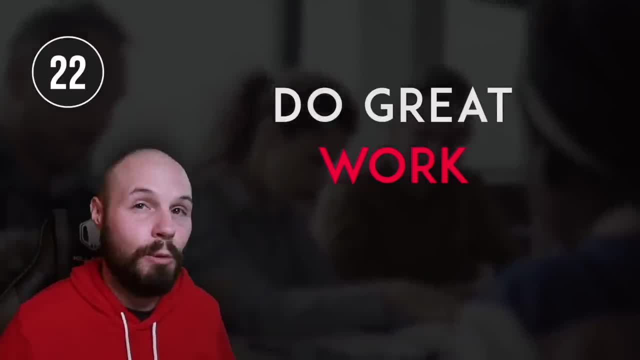 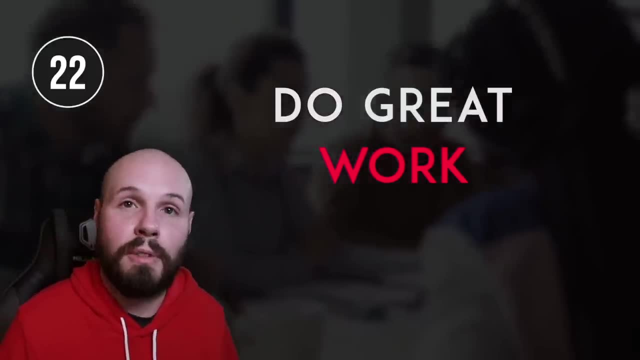 francisco or any other city. it's a small community. your reputation is a big deal, so at every stop, whether that's a contract or you know a company, do your best to put your best foot forward and impress people. number 23 is a common misconception. you're not too old. i started learning how to code. 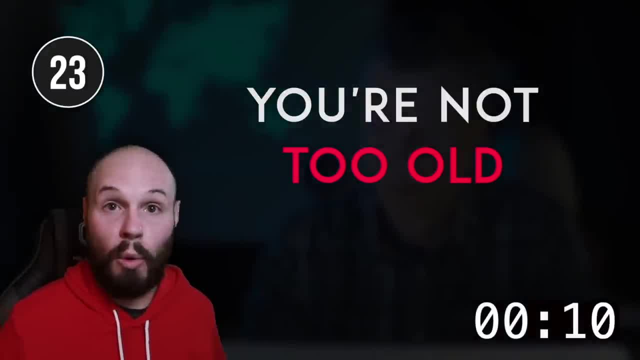 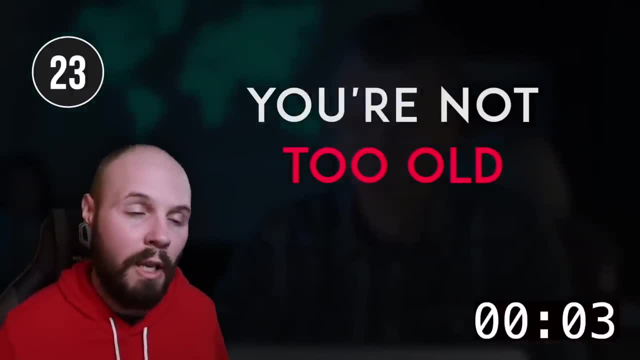 at 32 years old. i get questions from people all the time that are like 24- and i'm like 24, that think they're way too old, and i had this misconception as well. i thought you had to be a child math prodigy to be a computer programmer. that is not the case, and a lot of people are. 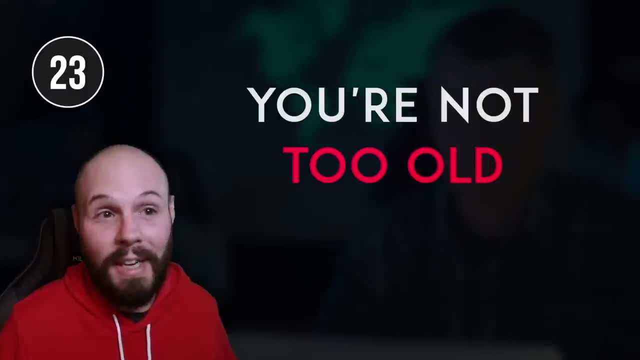 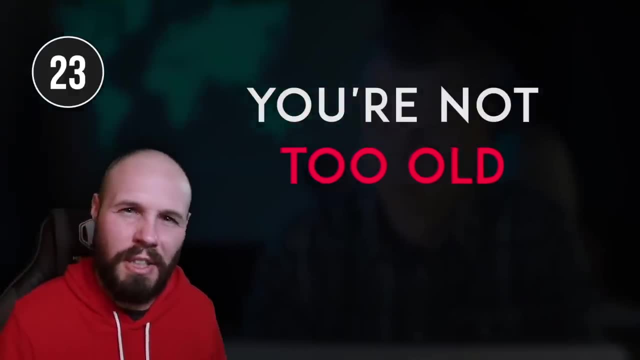 worried about like age discrimination in silicon valley? i don't see that. in fact, a lot of the engineers i work with are late 20s, early 30s, 40s, like it's it's. i think it's stereotypical to think it's for young people. it's really not number 24- another beneficial thing you can do for your 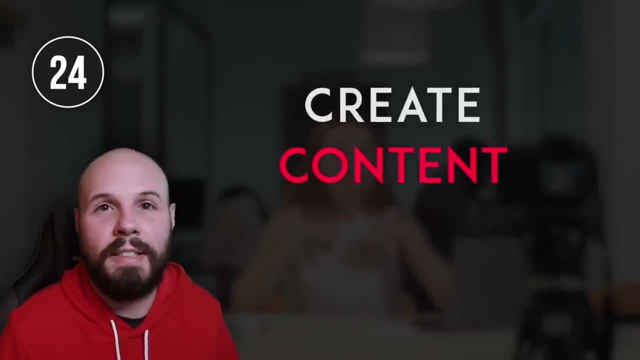 career if you can do it. this one's not for everybody, but that is to create content and build an online presence. that can be many things: that can be a blog, that can be a podcast, that can be youtube videos. you can just have a great instagram profile. having an online presence and kind of being known within your 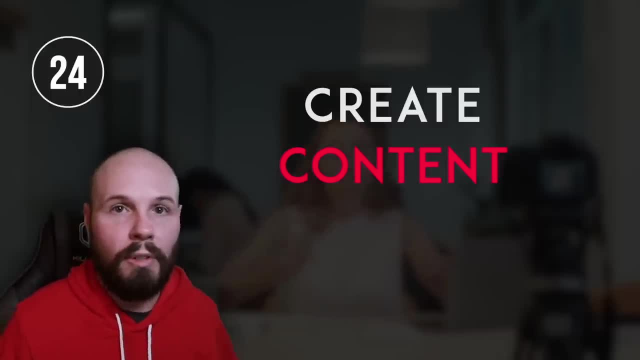 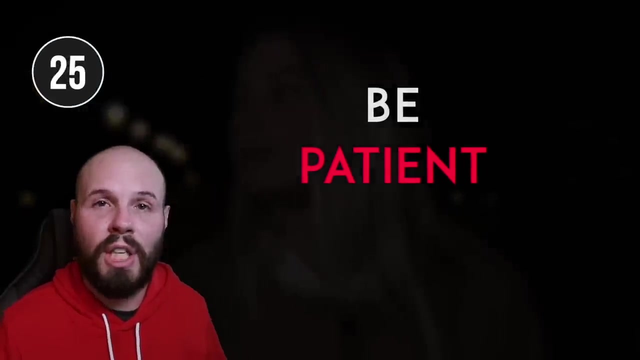 developer community, whether that's swift, javascript, whatever android, having that online presence and being known- hopefully known in a good way again- will benefit you. it's another way to network. you'll get a lot of opportunities if you become a known presence in your community. number 25: if you're still learning or trying to get that first job, be patient. this is a long 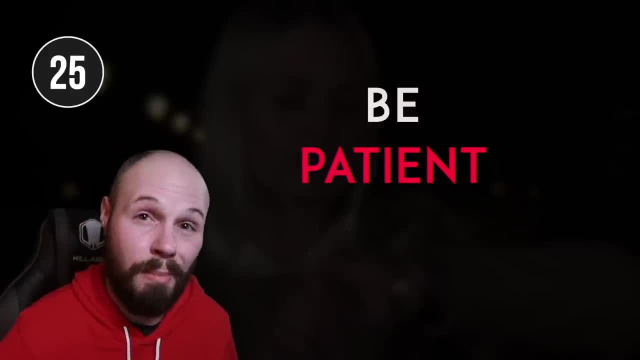 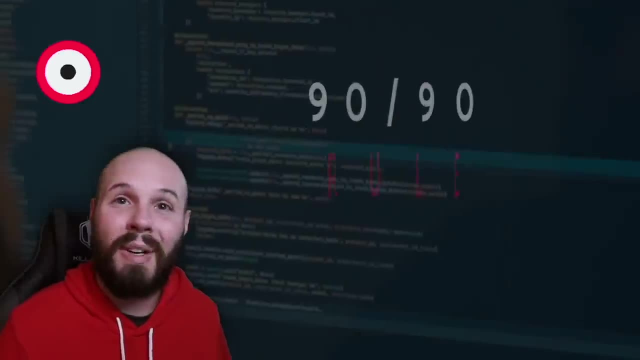 journey. so many people ask: how can i become a developer as fast as possible? that's the wrong attitude to have. this is a long journey, but i promise you it's worth it. at the end, number 26, let's talk about the 90- 90 rule. some people call it the 80- 20 rule. this has been called many 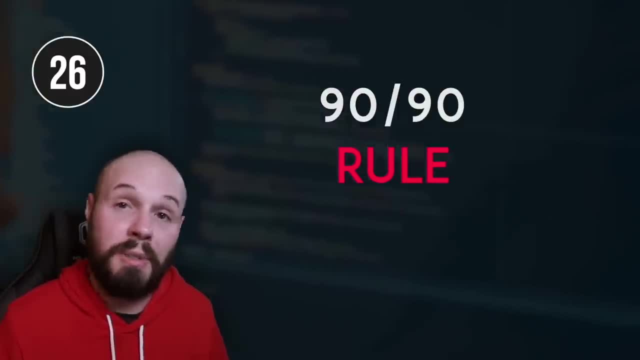 different things, but the point remains the same when you're building software. there's the first 90 and then there's the second 90. the first 90 is getting, like most of the features, done. it feels like it's so close to being done. the second 90 is all the air handling, the polish you know. 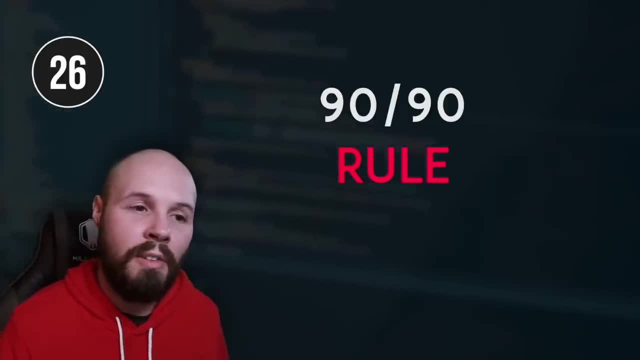 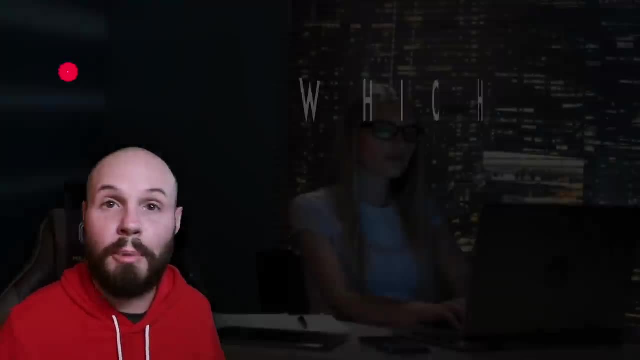 dusting for different screen sizes. you think it's a lot of little nitpicky stuff, but it really adds up into being like the second 90 of the project. it's a lot and it really sneaks up on a lot of junior developers. number 27: should you learn this language or that language? it doesn't really matter. 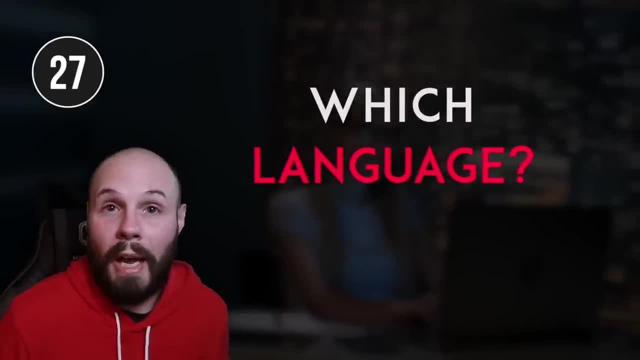 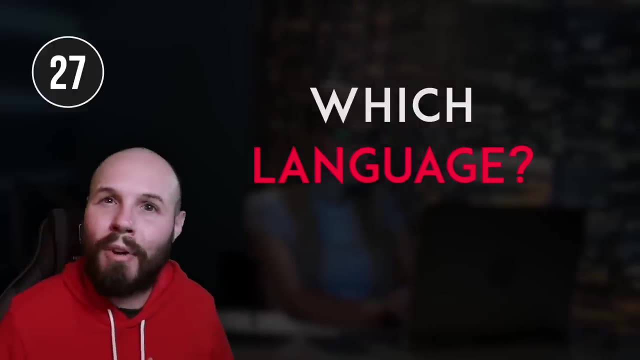 to be honest with you, if you do what you enjoy the most. my example: i enjoyed ios development. i like the iphone, so i wanted to build for that. if you do what you enjoy, uh, you're going to become good at it. most likely, if you ever have to switch languages, learning that second language is. 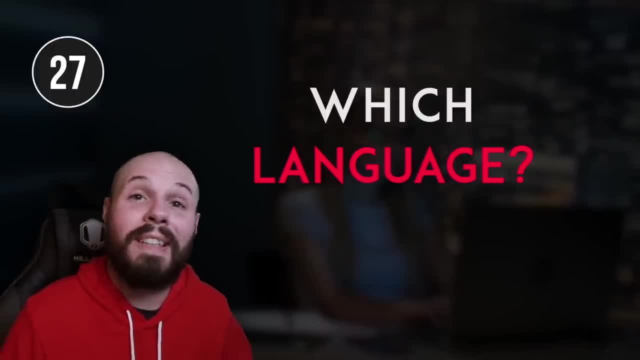 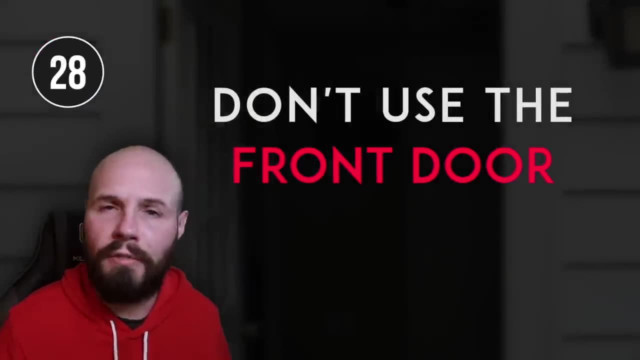 infinitely easier than learning how to program for the second language. so if you're learning how to program for the first time, so switching later on down the line could be relatively easy. if you have to do that, number 28, let's talk about getting job interviews. uh, don't go through the front door if 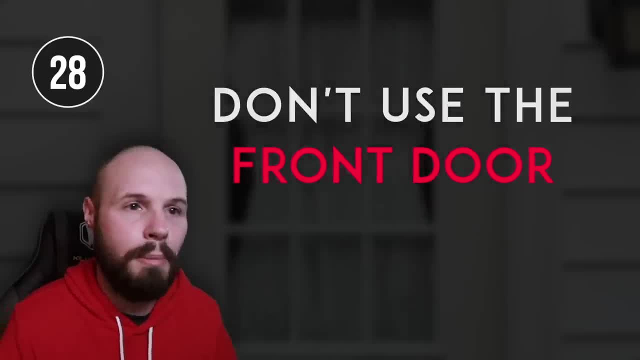 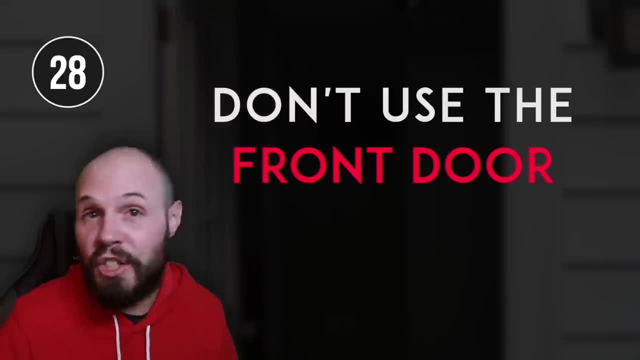 you don't have to. what is? what is the front door that is going to airbnbcom apply? uh, that's very hard to break through that way. again back to networking on twitter. if you start to get to know engineers at these companies, uh, build a relationship with them, dm them, say hey, can you? 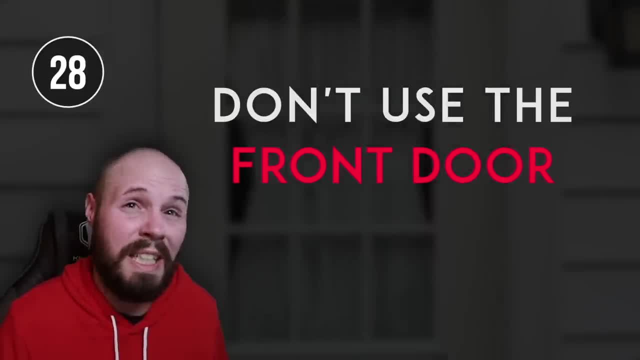 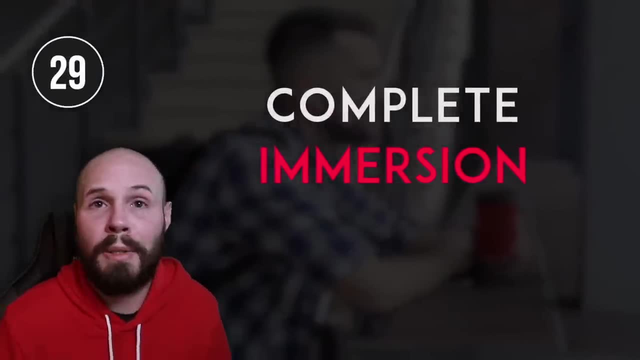 refer me for a job. most likely they'll say yes and that's pretty much a guaranteed interview. and then it's up to you. number 29: when you're learning, i suggest completely immersing yourself watching youtube videos, subscribing to newsletters, subscribing to blogs, just completely soak up everything you can. and along with that number 30, let's talk about 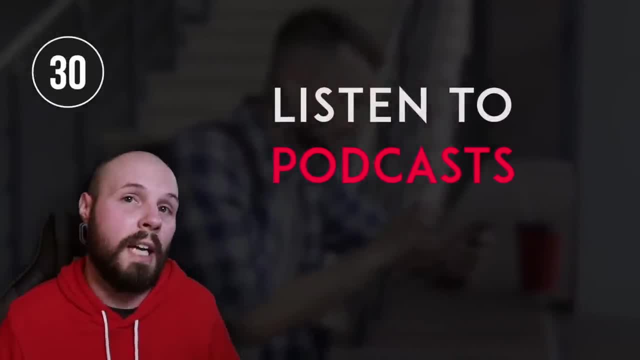 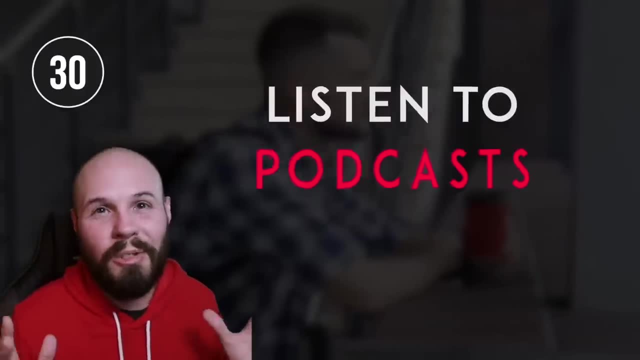 podcasts. podcasts are a great way to immerse yourself because you can multitask with podcasts. uh, commuting to work- throw on a developer podcast. going out for a walk- throw on a developer podcast. so podcasts are a great way to immerse yourself. number 31: when it comes to getting contracts, when 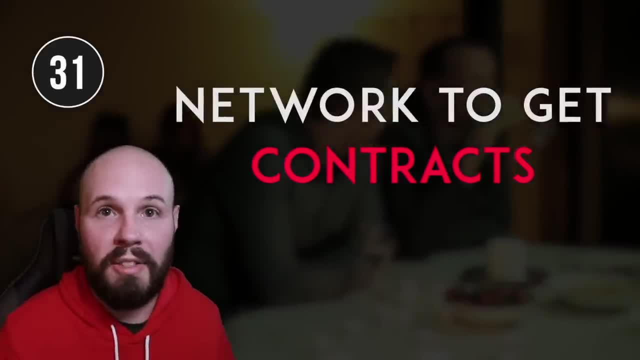 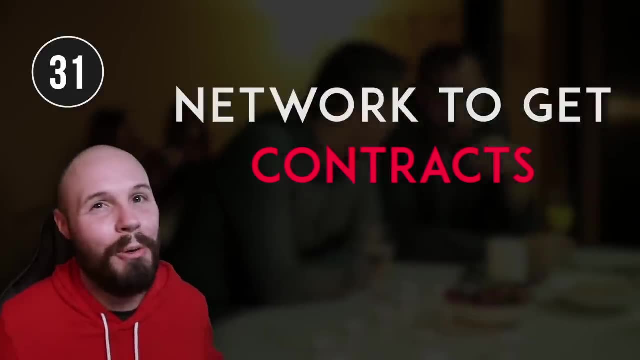 you're ready, your personal and professional network will be the best, and by best i mean getting opportunities, but also getting a job. you're going to have a lot of opportunities to get, but also getting quality opportunities going on sites like upwork. you never know what you're. going to get. you could get some really crappy projects, but if you're recommended by a friend or a former co-worker to another company, those are going to be quality contracts and that is how i've gotten all my contracts- number 32- should you work at a small startup or a big company? 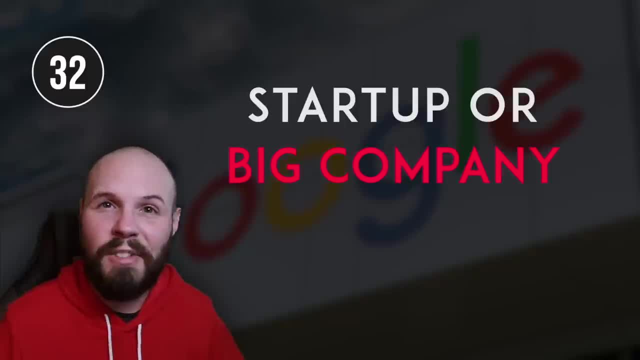 as with any programming question, it depends. if you like to wear many hats, you consider yourself a generalist. you want to build the whole app or the whole website, that's a small startup. if you want to work on a very large team, on a large company and 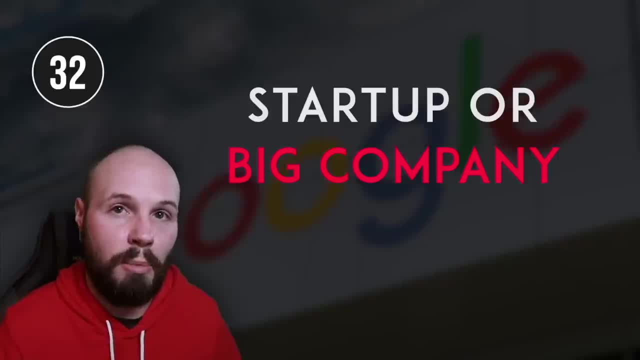 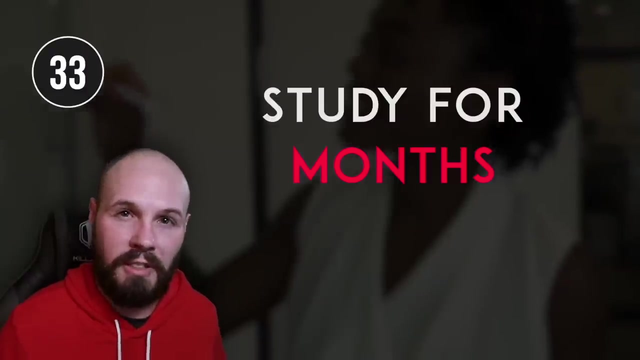 be very specialized. that's a big company, so your personal preference comes into play also. obviously the larger company, probably a larger paycheck, but maybe more stressful. smaller startup- uh, smaller paycheck could be less or more stressful, it depends. number 33: preparing for job interviews- big tip: it takes months to prepare for these data structures and algorithms. 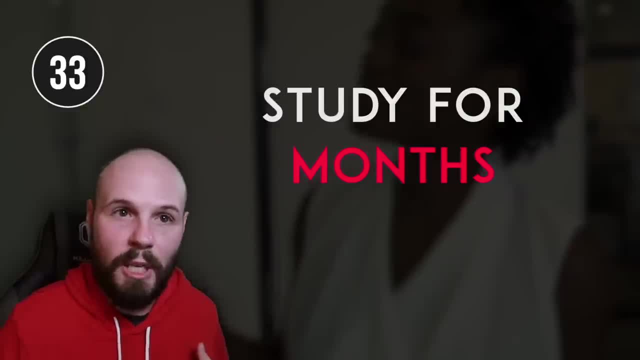 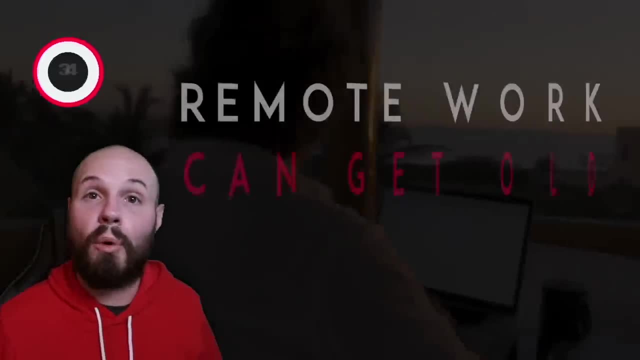 questions: practice, practice, practice, practice. what i've done in the past that has messed me up is two weeks before the interview. i'm like, okay, i'll start studying. that is not enough time. give yourself a couple months, not a couple weeks. number 34: remote work has its downsides, right, it's the dream to work wherever you want, whenever you want, remotely. 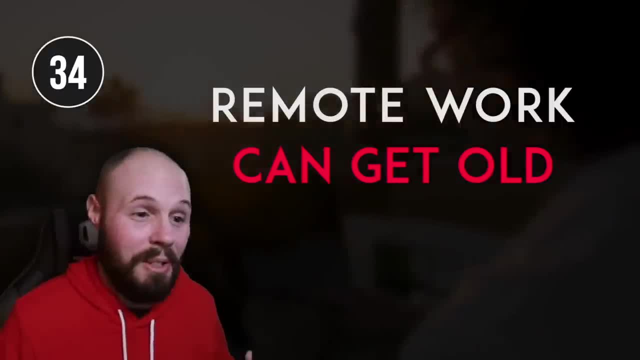 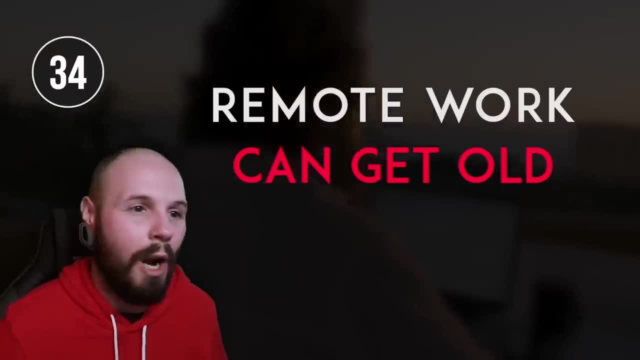 uh, that sounds like the dream. but and it is fun for like six months, like the honeymoon period, after doing it for a year or two, it really starts to have its drawbacks: the loneliness you're by yourself most of the time, not working with people, and again, that may sound great, but after a long 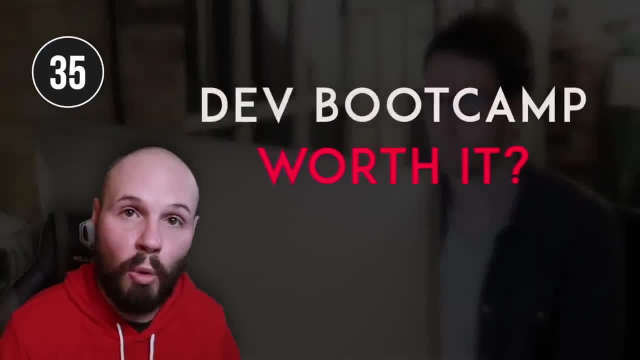 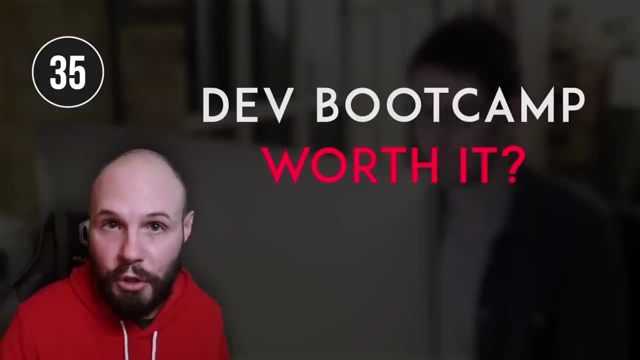 time of that, it starts to wear on you. number 35. is a dev boot camp worth it? uh, what i have found, the knowledge you get? no, it's not worth that 10 000 potentially, however, forcing you to do it every day for eight to ten hours for x amount of weeks, getting the experience of working with other. 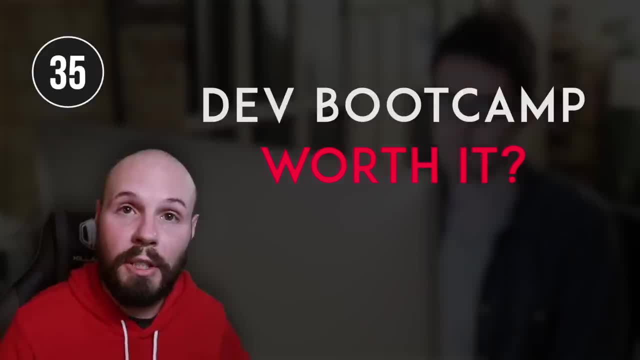 people. that is absolutely worth it. so if you think you can be a good self-starter and learn on your own, i think you should probably save the 10 grand. however, if you like the extra push to force yourself to do it for eight to ten hours a day, i think a boot camp is worth it. and number 36 after: 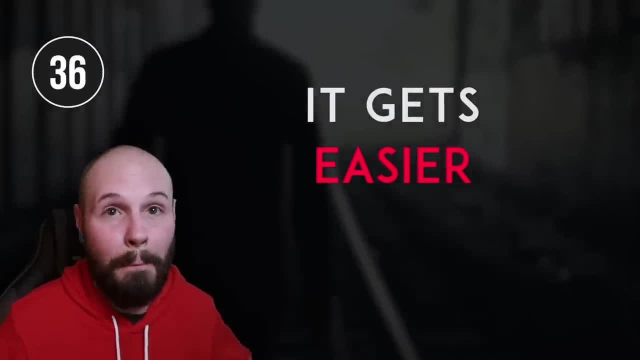 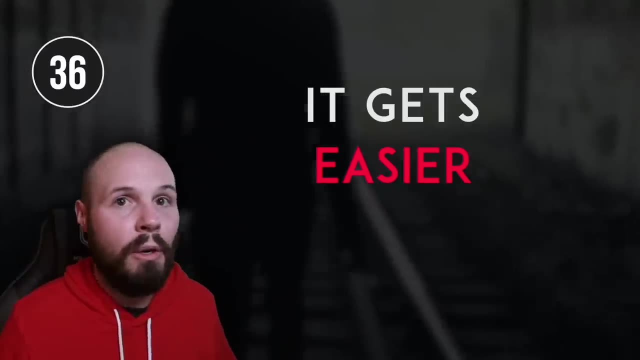 all these tips, it gets easier, like experience in this industry matters, right? this may have been an overwhelming video throwing a lot at you, and i know you may be learning, and it may feel overwhelming, but before you know it, you're going to want to get started and you're going to want to 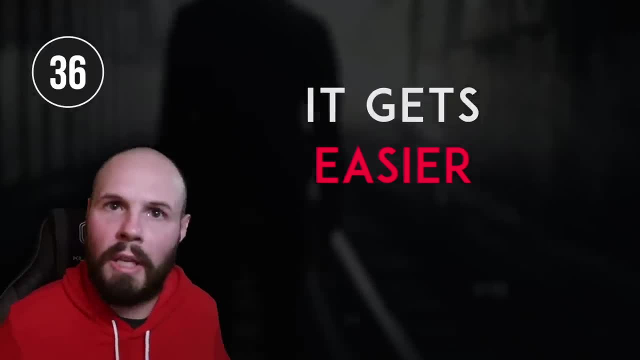 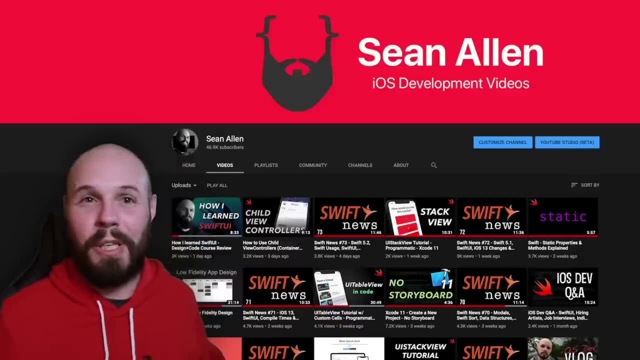 wake up and five years has gone by and you're like: holy crap, i know a lot of stuff now, so it does get easier. stick with it, i promise. and, of course, number 37 is to uh, subscribe to this youtube channel or any other developer youtube channels. again, immerse yourself. i put out ios. 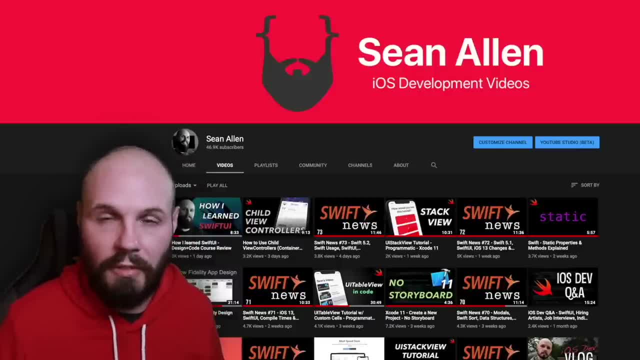 development content specifically, but i do talk about general software engineering stuff a lot as well. so those are my 37 quick tips. i hope you got something out of this. let me know in the comments. if you disagreed with anything, let's have a discussion. we'll see in the next video. 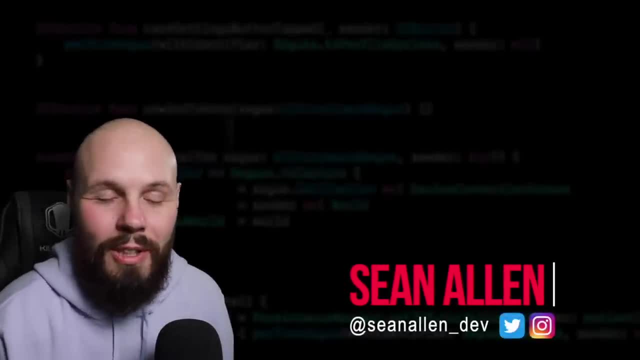 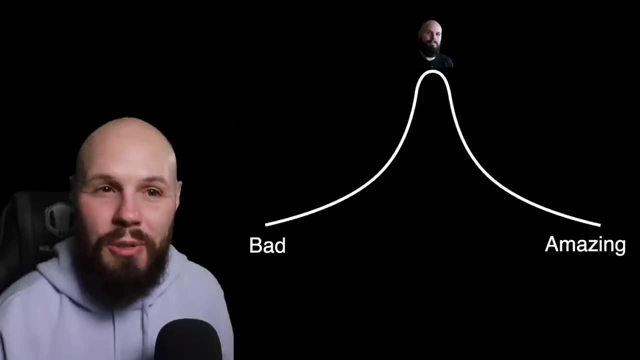 when it comes to my technical skills, i'm an average developer, like if there was a, there was a normal distribution bell curve, i'd be parked right at the top of that thing. right, i'm not great, nothing special, but i'm not bad either, just average. however, i think i'm a really 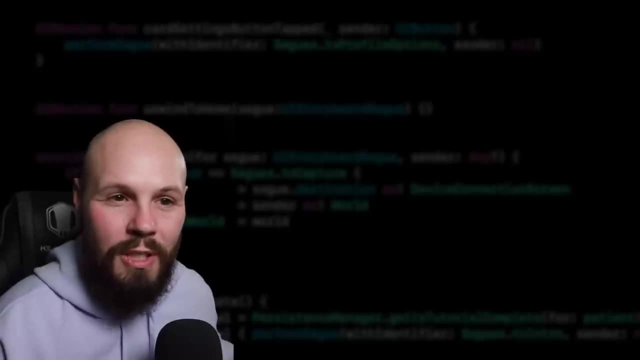 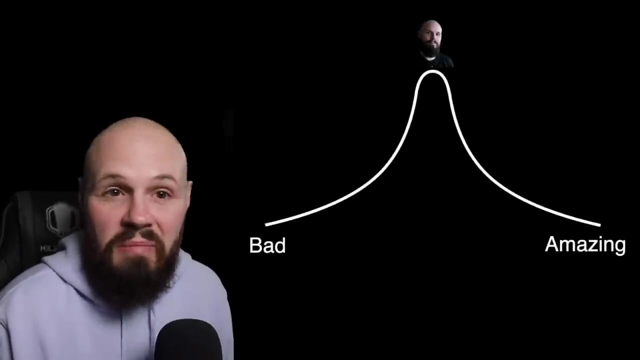 good developer overall, and that's what we're going to talk about in this video, because i want to maybe dispel some misconceptions that are out there. so, like i said, my technical skills they're fine, right, nothing special, not bad, just just average. however, i think there's a misconception. 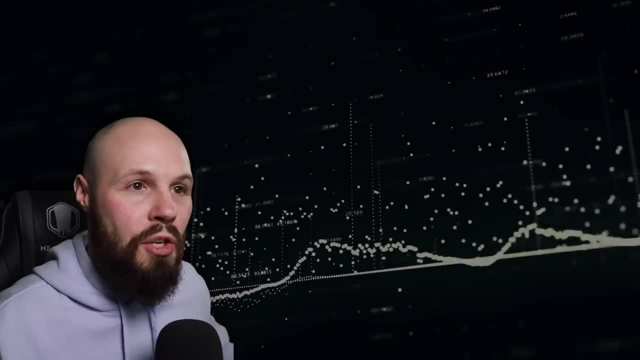 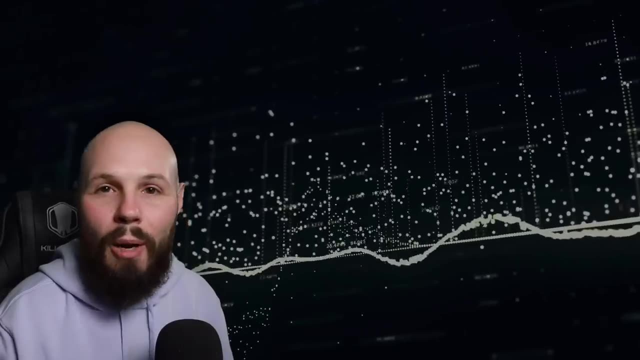 out there, probably because i create content and put out a lot of stuff that i just know so much. and again, this is the misconception that i want, i want to dispel right, because i get dms emails, you know, comments on youtube asking like very specific questions about all kinds of frameworks. 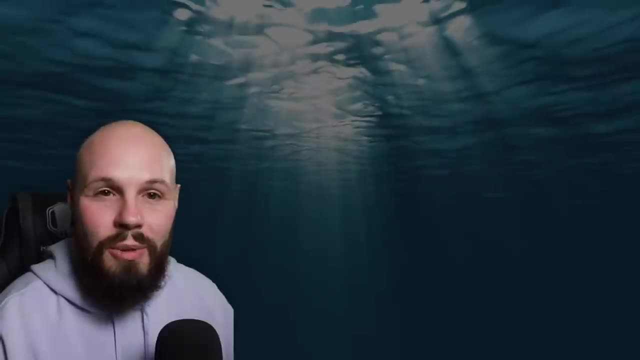 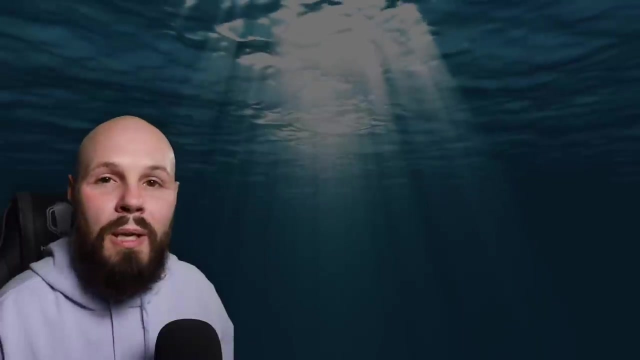 and then, as you know, like there's a whole ocean of knowledge that you can have, like it's impossible to know everything about everything. and again, this is the misconception that i want to hopefully dispel in this video: the more experience i gain, the more i realize that, like i don't 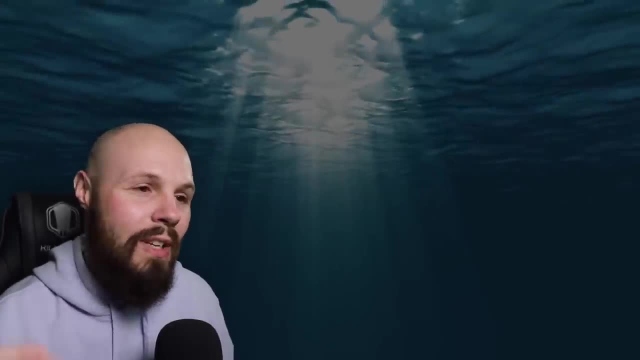 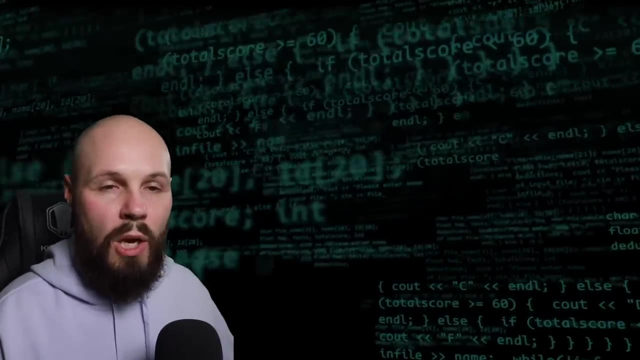 know much and there's a difference between knowing something, like having it memorized, versus being able to figure things out quickly and being a quick learner. and again, this is the misconception that i want to dispel, because i know a lot of you out there are probably just. 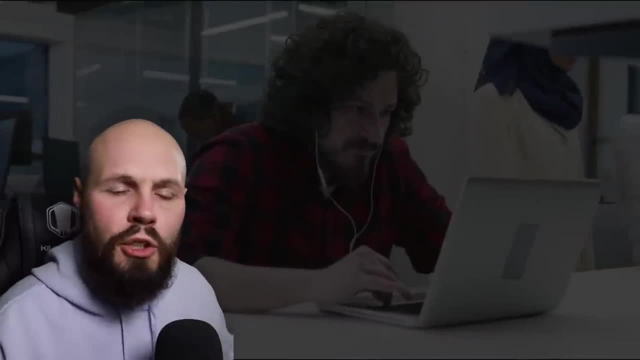 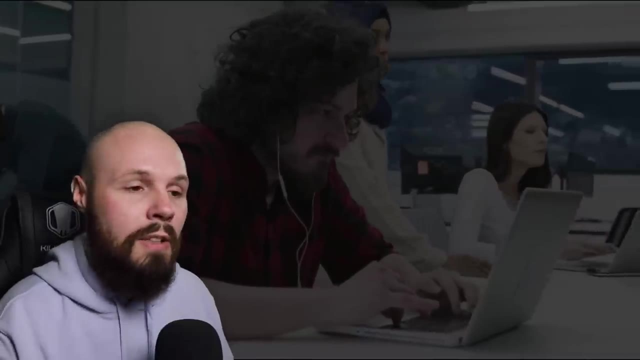 learning, software development or just learning swift, or you're earlier in your career and you're probably very self-conscious about your, your knowledge, right? you probably look at these developers on twitter or content creators and you think to yourself like, wow, i don't, i don't know. 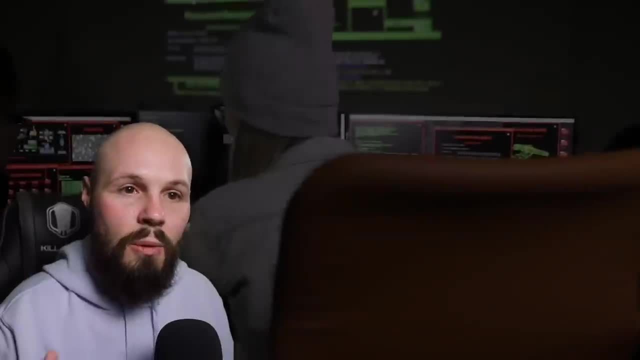 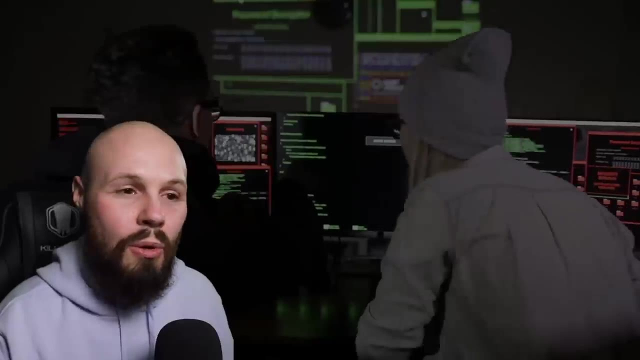 nearly as much as they do, and you're self-conscious about your knowledge. well, again, i want to say that, like you, don't have to know much, but there's a couple keys. even if your knowledge is mediocre or less, there's some things you can do as a developer to make yourself. 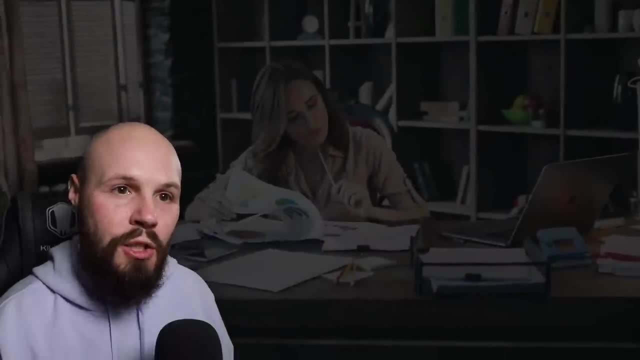 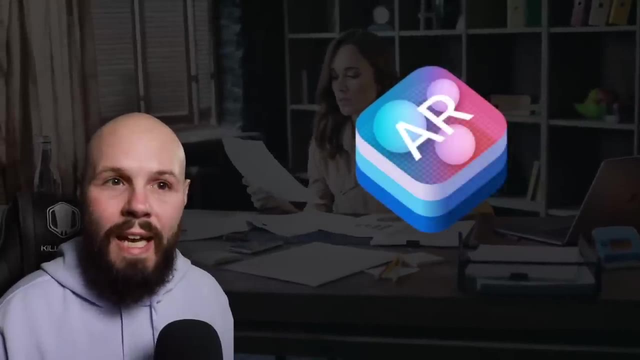 really, really good, and i alluded to one of those just a little bit ago, and that is your ability to learn. like i said, i don't know much off the top of my head like ar kit, for example. i don't know anything about that. however, i'm confident if i were to get tasked with building an ar app like 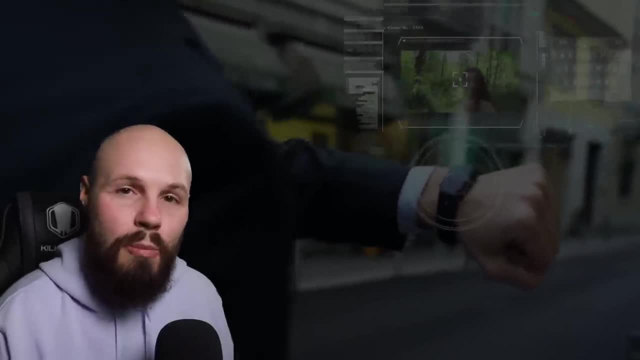 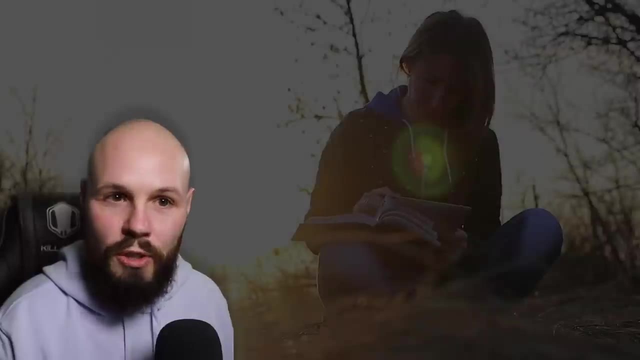 i would dive into the documentation, i would read books like. i'm very confident that i would be able to pick up that knowledge and skill set relatively quickly. and i think that's the big thing is learning how to learn, whether you learn by reading books or watching videos or diving into 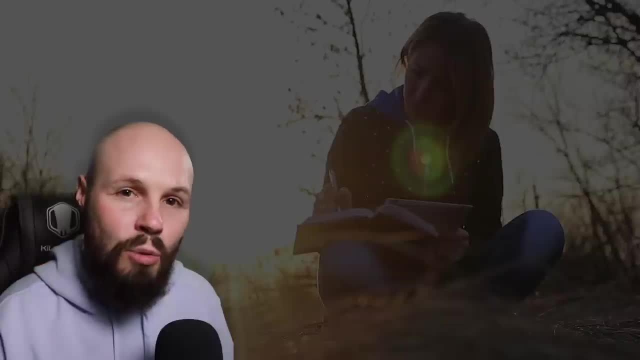 documentation or listening to podcasts like figure out how you learn, because the ability to pick up new skills and new knowledge relatively quickly is a huge part of being a developer. you don't have to have every framework out there memorized and, besides, learning how to pick things up quickly, 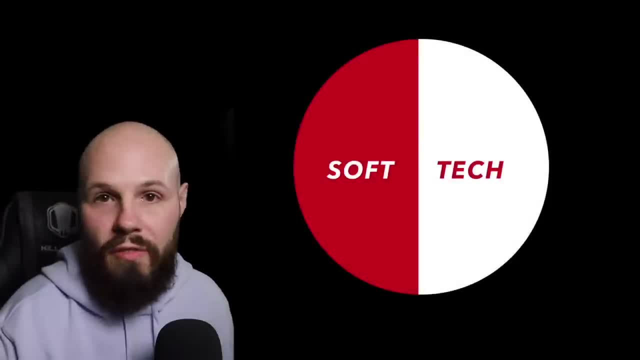 there's a whole slew of soft skills that i believe are at least half of the equation right. there's skills and then there's your soft skills, and that's where, even though i say my technical skills are average, i believe my soft skills are way, way, way above average, and that's what i think. 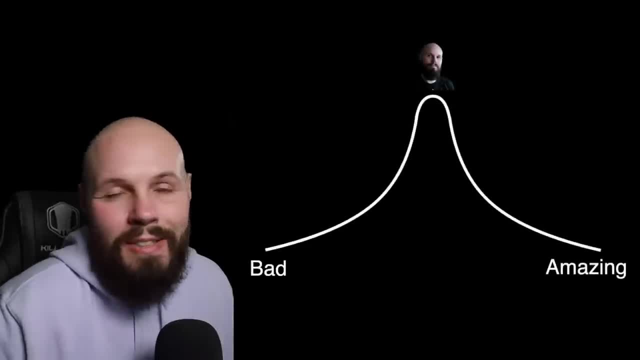 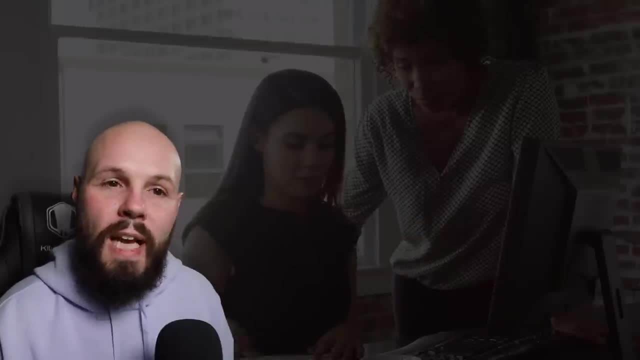 makes me a good developer overall, even though my technical skills, like i said, are just, they're fine, they're average, and those are skills that you can work on right, like your communication skills, like having the ability to break down complex technical topics, not only to maybe more junior developers or 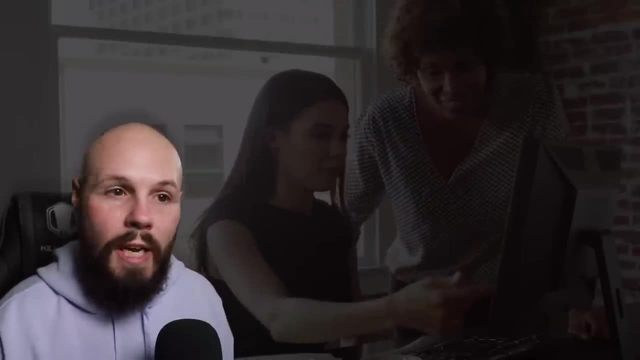 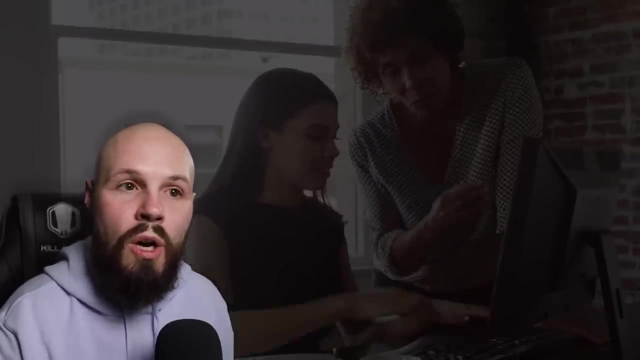 other technical people but other non-technical people at your company or on your team, for example. so i'm constantly having to communicate to you. know the ceo, you know the trade-offs, uh, between how complex we want to make this feature right, because what happens with you, know marketing and product. 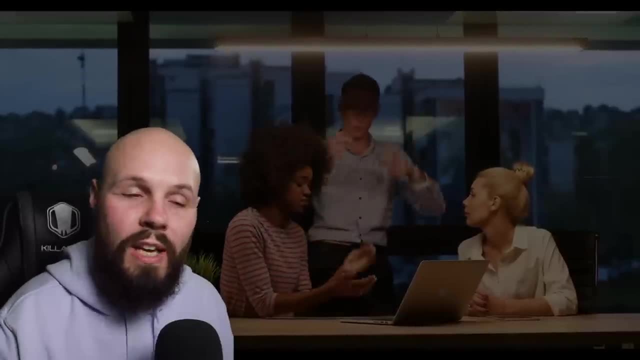 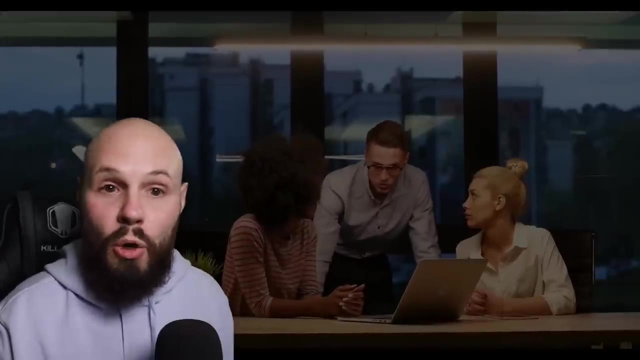 people, uh, or co-founders- like they want to add features, add features, add features. well, it's up to you as a developer to properly communicate. like hey, that's fine, we can add this feature, but you know, we're either going to have to get rid of another feature or make some trade-offs because 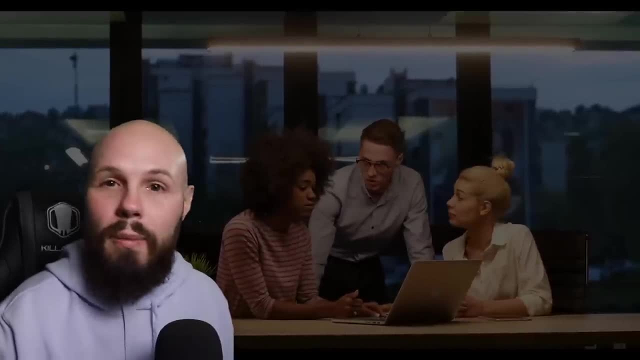 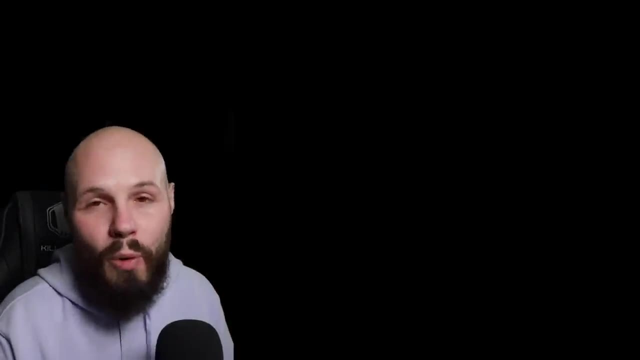 we have a launch date that we got to hit and if we keep adding features, like we're going to miss out on some of those features or we're going to lose some of those features or we're going to lose some of those features, and so communicating that and having those discussions is an insanely. 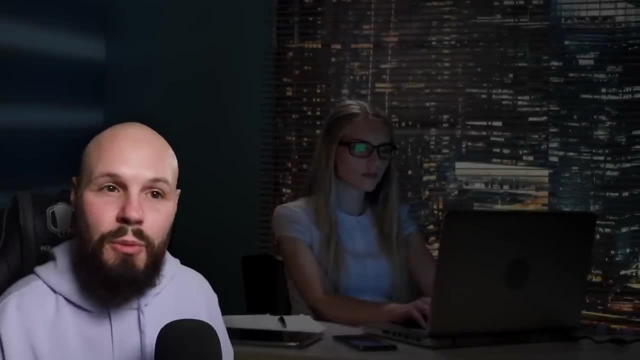 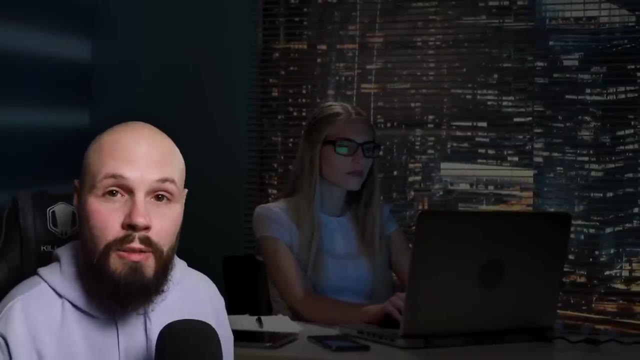 valuable skill for a developer. and, of course, the number one thing you can control is your work ethic. right, you can just be a hard worker, back to that ability to pick things up quickly, you know, diving into books, learning new things like that work ethic and that drive like you can control. 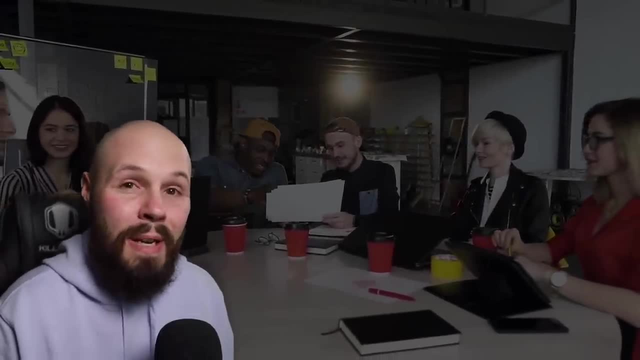 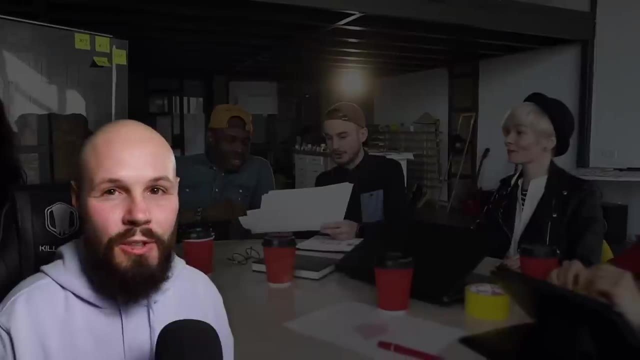 that you can. you can improve on that and then other soft skills, like the passion you have for your job and your craft, also being a good teammate. like it doesn't matter how great of a developer you you're bad to work with. like you're going to be a net negative on your overall team, no matter how. 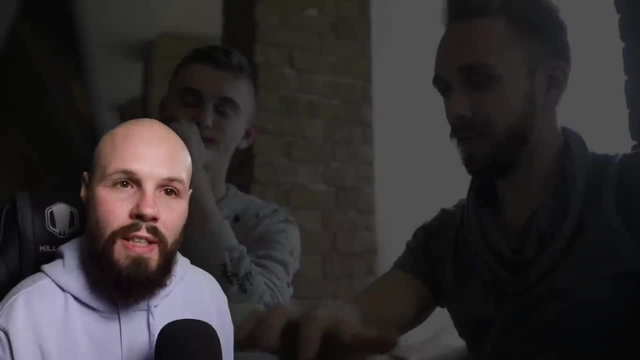 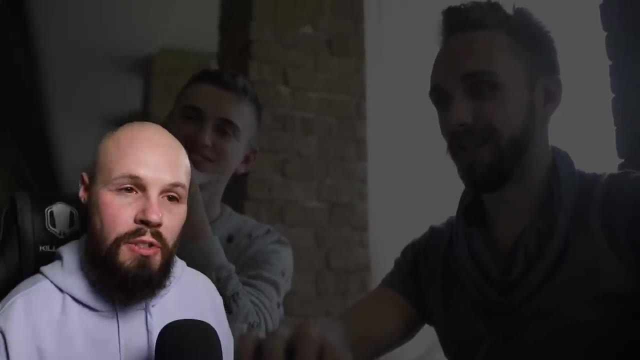 good, your skills are. another soft skill you can work on is showing initiative. like right, like don't always wait and sit back and be told what to do. now i'm not saying go rogue, but if you're a junior developer, like go to your senior developers or go to your team and say, hey, i 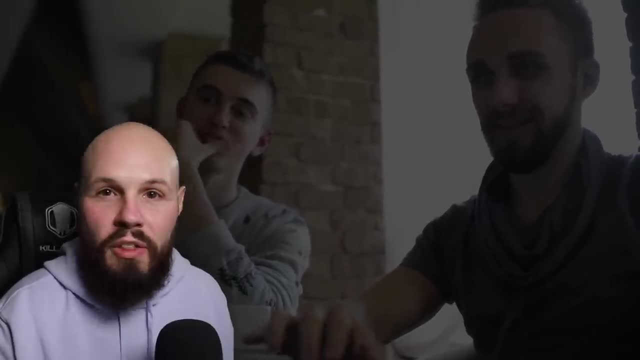 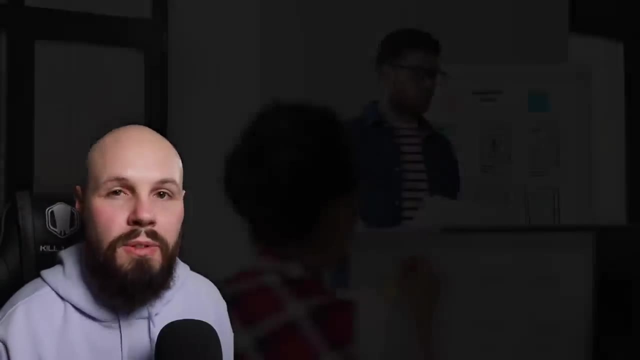 had this idea. i want to research it. i want to look into building this. what do you think you know? and showing the initiative will go a long way towards making yourself a more well-rounded developer if you feel like you're lacking in your technical knowledge. and then, of course, you can. 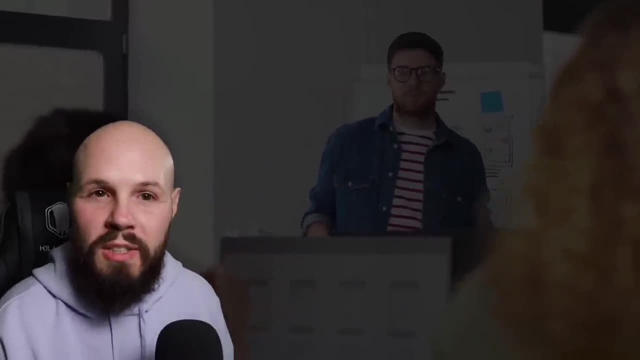 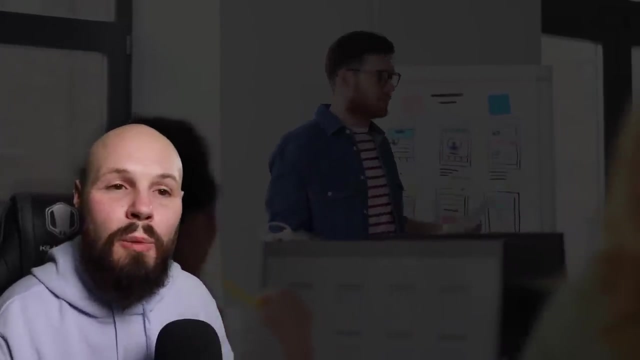 start researching uh, ui ux, design, overall product stuff. again, because, this is right, we're talking about making up for a lack of technical knowledge. well, again, there's a lot more that goes into being a developer than just knowing the code right, understanding, like i said, the ui ux, the product. 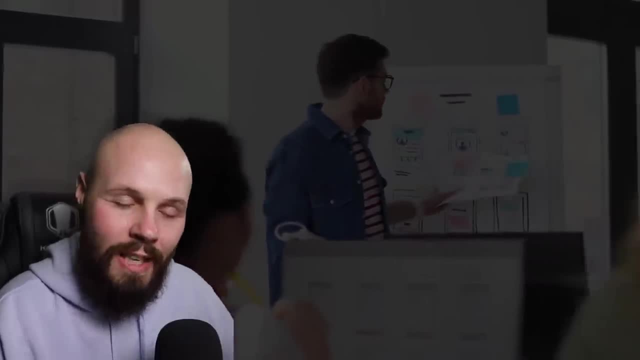 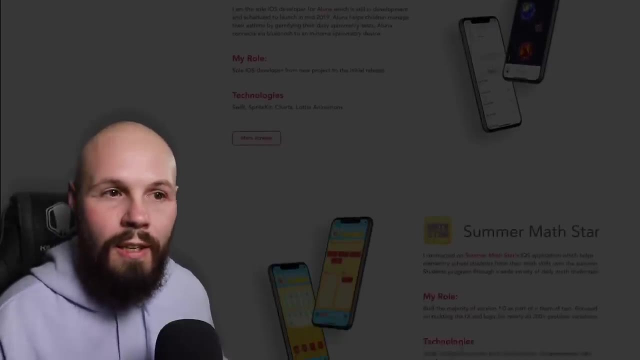 design, like start studying that, start getting very, very good at that, because again that makes you more well-rounded. and then, lastly, when it comes to getting that job, or getting the next job or winning that contract- like the ability to market yourself is such a big deal- and having a great 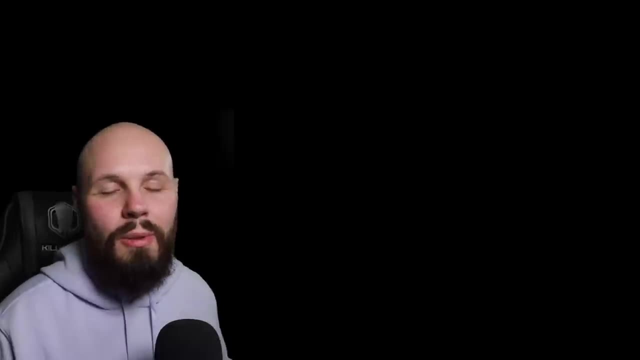 online presence and developer portfolio really goes a long way with that. so, again, i consider myself an average developer when it comes to just straight up technical skills, and if you feel that way too, or you feel self-conscious about your technical skills, of course you can still work. 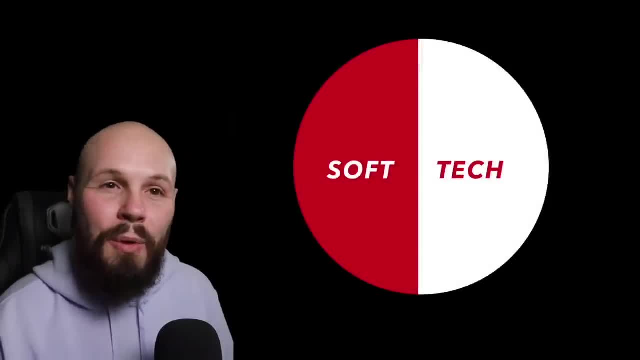 to improve them. i'm not saying you have to know nothing and not work at that, but there's many other things you can do, like the soft skills we talked about and learning how to learn. learn how to pick up things very, very quickly, uh, to kind of make yourself a more well-rounded developer. 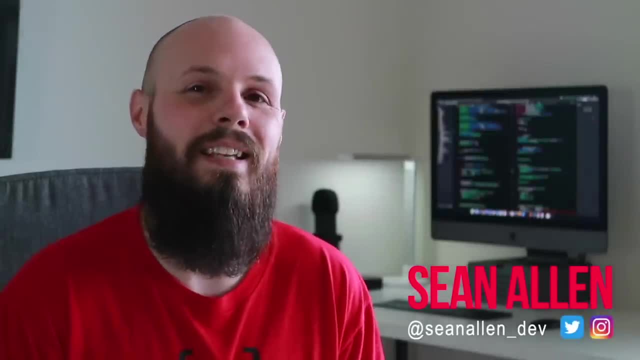 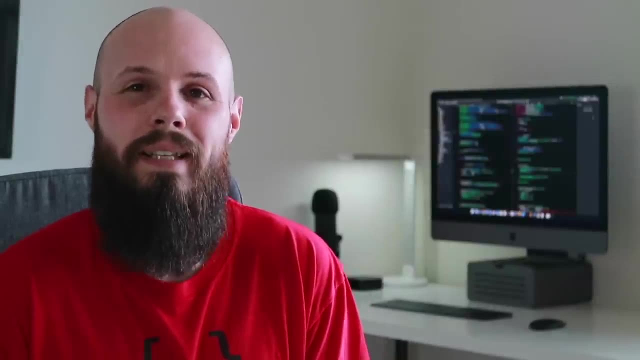 what's going on? everybody sean here today we're going to talk about nine things that i wish i knew when i started out. programming uh would have saved me so much time. so let's just dive right into the list, and the first thing that i would recommend to my former self is to not stay in what i call. 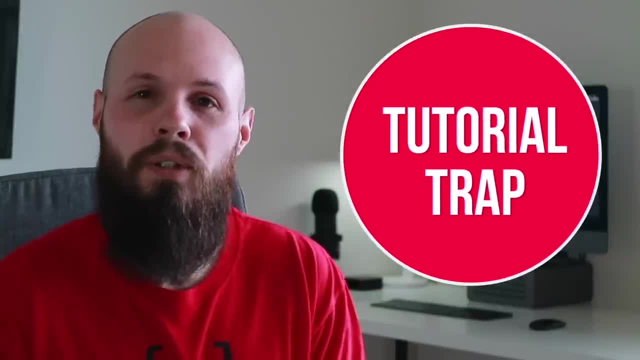 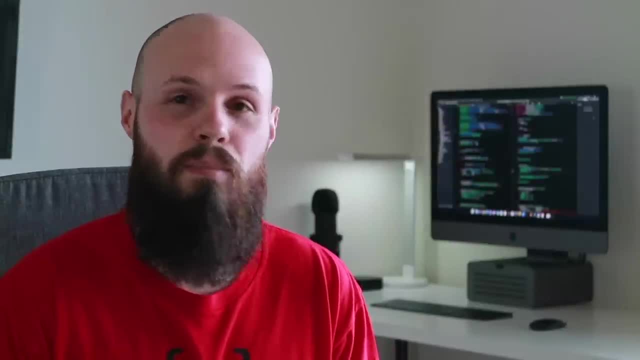 the tutorial trap for so long. what is the tutorial trap? well, i think a lot of us fall into this, where we just enjoy learning. right, we like learning new things. so we see this bright, new, shiny toy and it's like: oh, let me do a tutorial on that. and 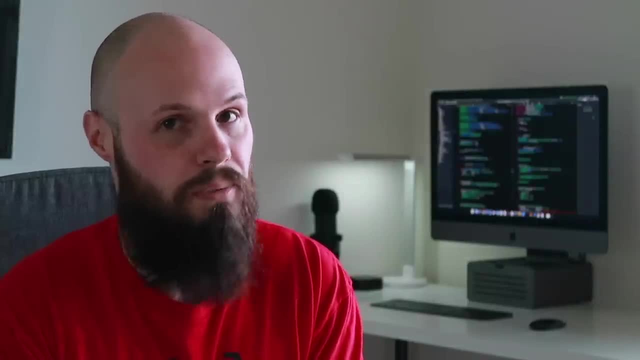 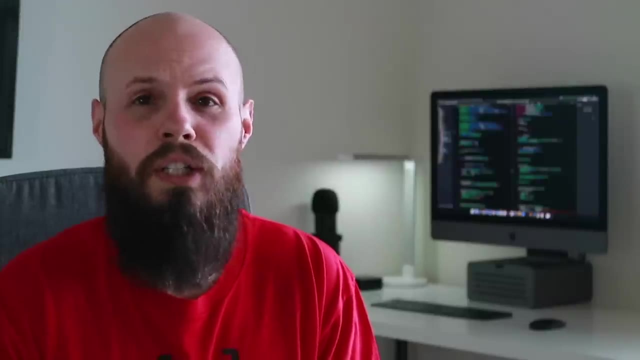 when you're just learning. don't get me wrong, you have to start out on tutorials. that's how you learn, right. but uh, what you may find yourself falling into is just tutorial after tutorial after tutorial. you've been doing that for six months and you haven't built anything on your own. 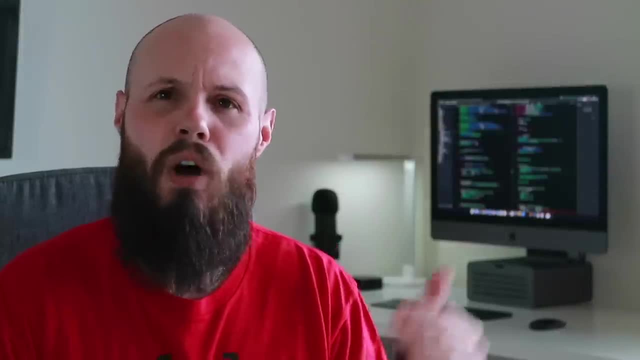 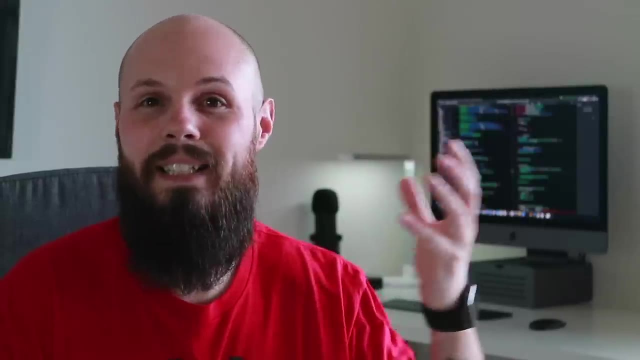 when i decided to build my own app, my own idea, where i couldn't just follow a recipe of a tutorial like a to-do list, a paint by numbers, my learning skyrocketed. you know, i was forced to take the ideas in my head and make them happen on an app. right, i wasn't following somebody else's. 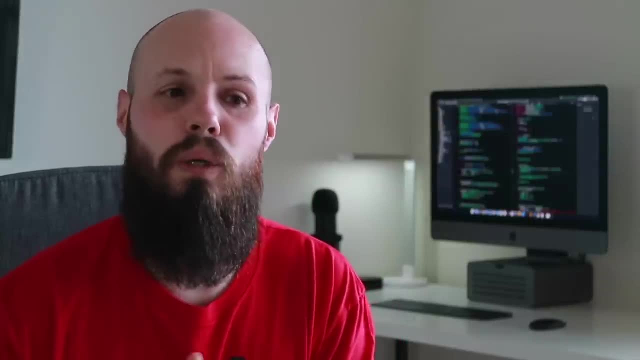 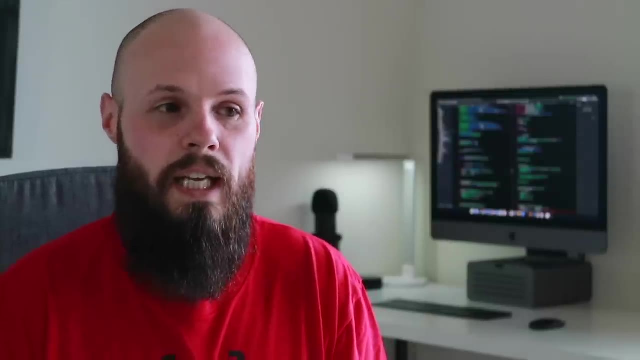 so i had to dive into the documentation. or maybe i did follow a tutorial, but i could only take bits and pieces from it because it wasn't you know exactly what i needed. uh, anyway, long story short, if you find yourself in this tutorial trap and feel stuck, like you can't build anything on your 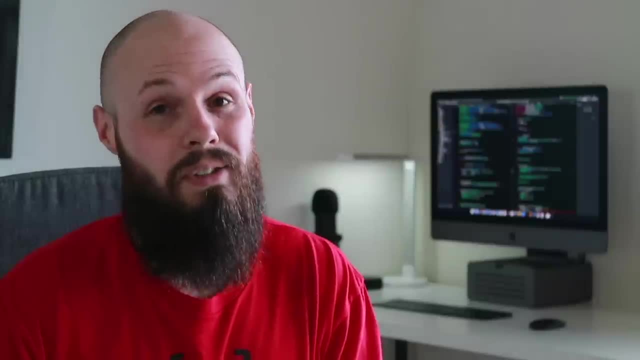 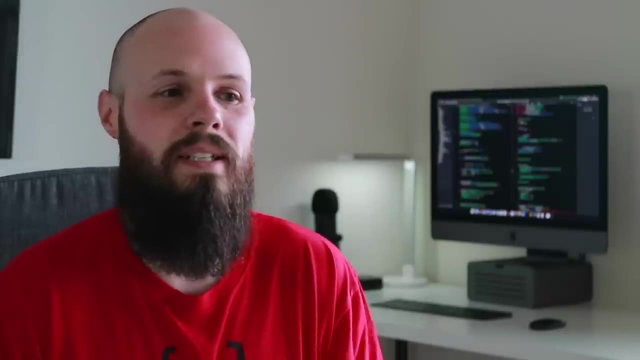 own. you have to follow a tutorial. the only way out of that is to start building stuff on your own. it's going to be rough at first, but trust me, your learning will go through the roof. the next thing i want to talk about is to- not, you know- skim over the fundamentals of the language. to move on to the 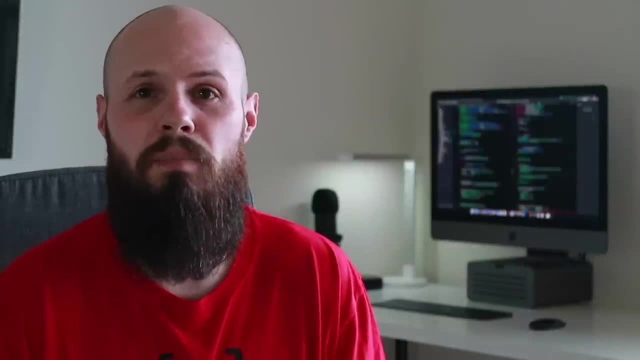 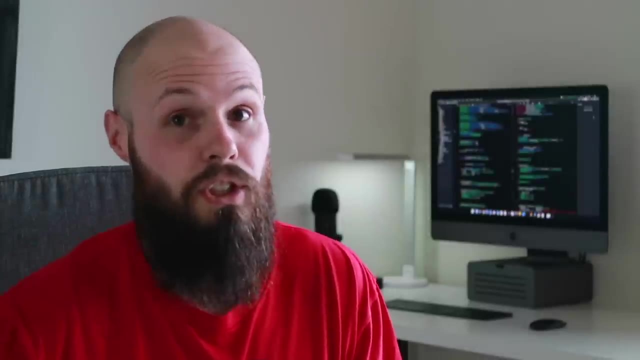 will, right, really drill those fundamentals. it's like. it's like playing a sport, right. if you're, if you're trying to learn how to shoot a basketball, you're going to shoot thousands and thousands of shots. you're just not going to go right into playing a game. well, you shouldn't go right. 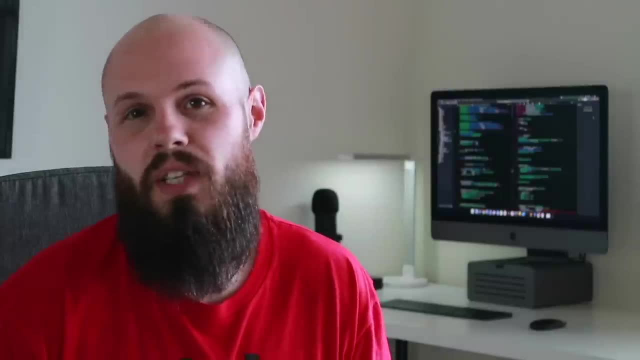 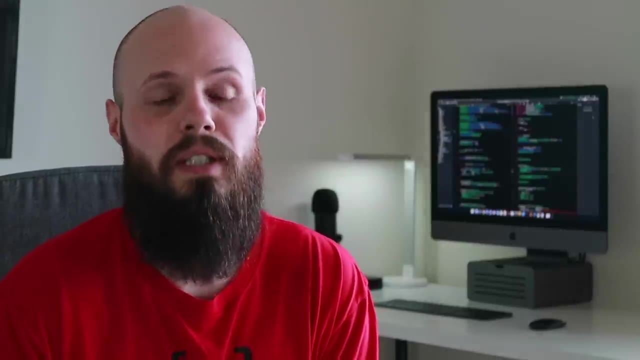 into playing a game when you've only shot a couple shots, right. so same thing with the fundamentals of not only the language, but of, you know, ios. speaking from an ios developer specifically, like i use table views as an example. you can't just build one table view and think you're good to go on table. 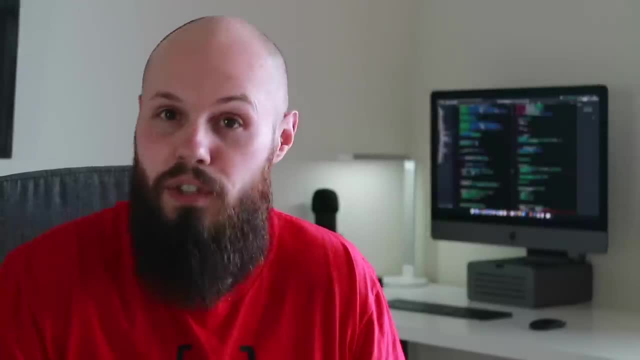 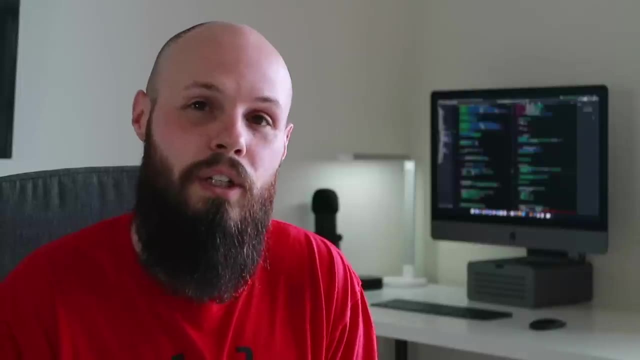 views onto the next thing. right, you just got to drill it. it's like shooting a thousand jump shots. i know table view so well, it's because i built a thousand of them. right, you're not just going to build one and then know it cold. so drill the fundamentals not only of the language, but of 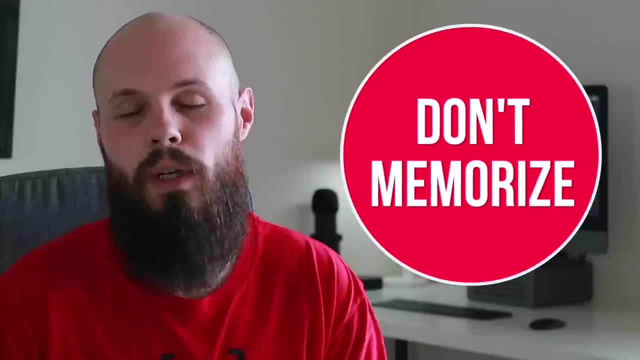 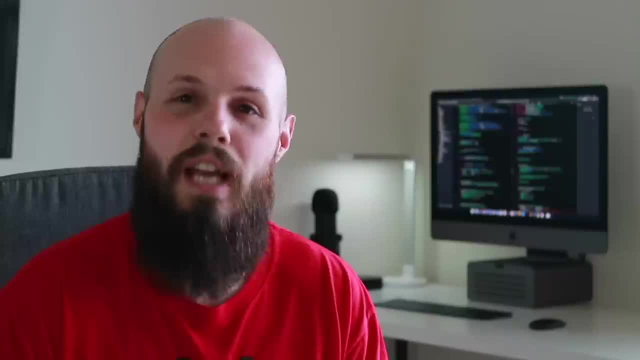 the platform as well. my next piece of advice would be to not worry about memorizing things. it doesn't matter how senior of a developer you are. you're probably going to google the simplest of things each and every day, like it just happens to all of us, the. the key here is to know where to look for. 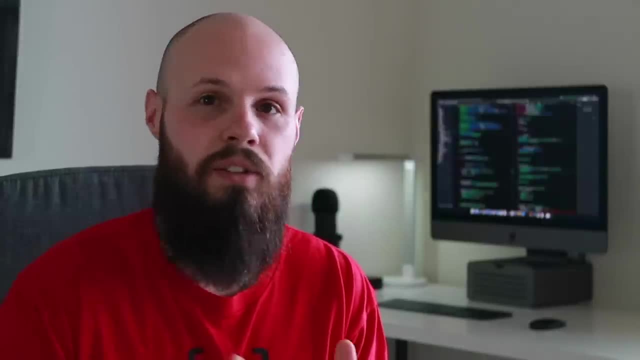 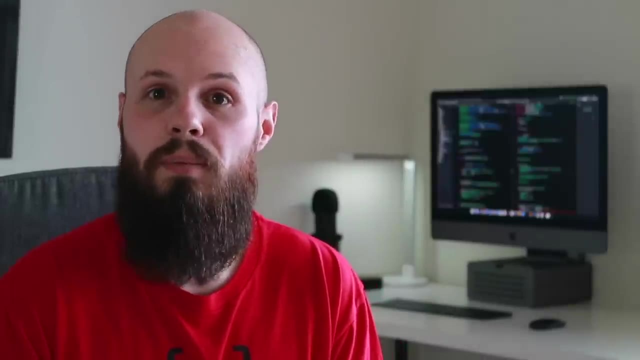 where to find the information you want, whether that's documentation, a certain blog post, etc. but don't worry about you know being able to. i- i think people starting out have this misconception- that senior developers just sit in front of their computer, just type away, you know, for an hour without looking something up. 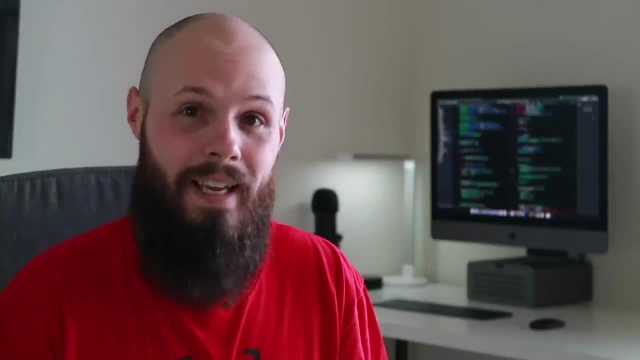 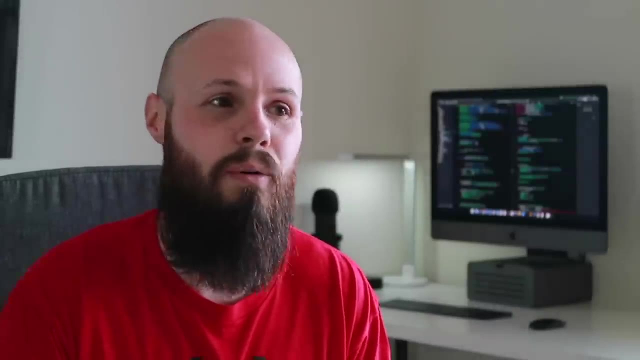 they just do it all from their head. that is absolutely not the case. i mentioned table views earlier, even though, sure, i can create the pretty typical standard table view. but if you do anything with like dynamic cell height or maybe section headers, that kind of stuff, i'm gonna be like oh, 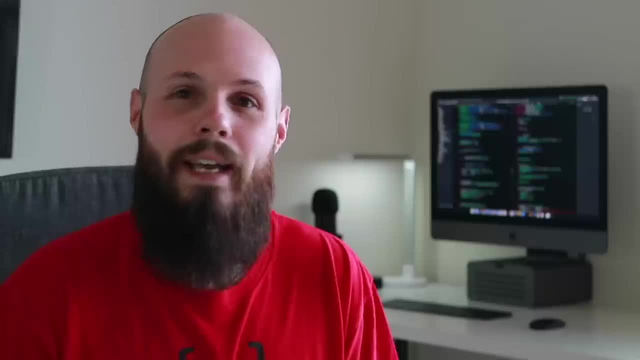 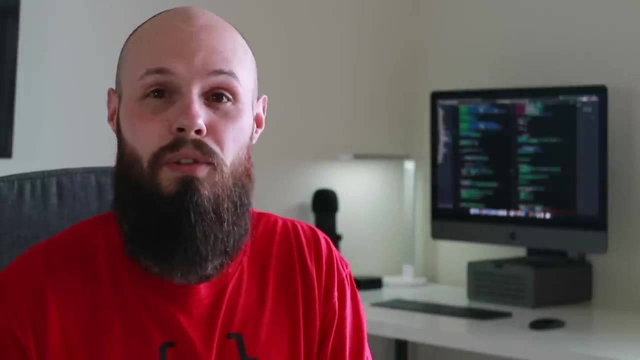 you know, i can't remember how to do that exactly. let me look that up real quick again. you have this kind of thing where you can just type away for hours, never looking anything up. couldn't be further from the truth. so the key here is to kind of learn how to learn and then also like know where. 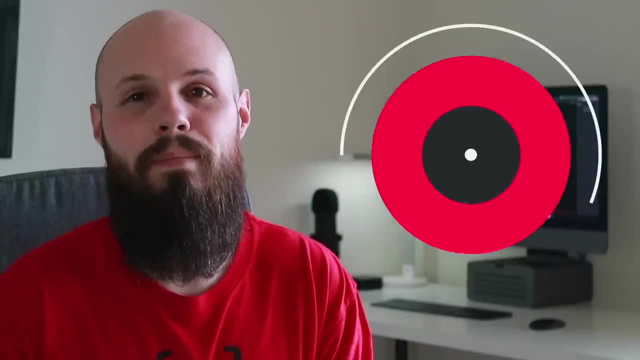 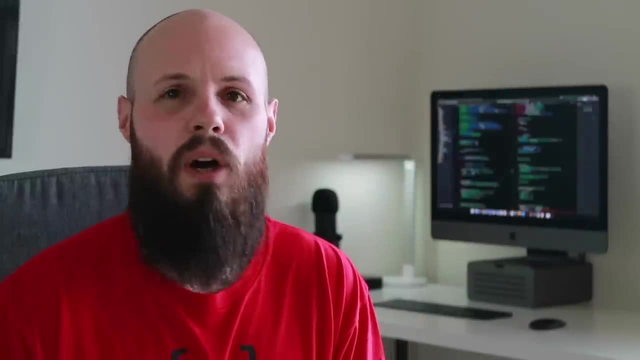 to find this stuff. don't worry about memorizing. next up, i want to talk about finding a mentor now. this doesn't necessarily have to be somebody in person, you know, if you live in a remote place where there's not a lot of developers. it can be online via twitter, etc. or online coaching some. 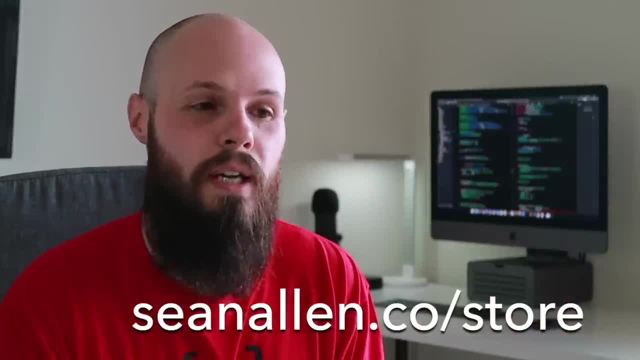 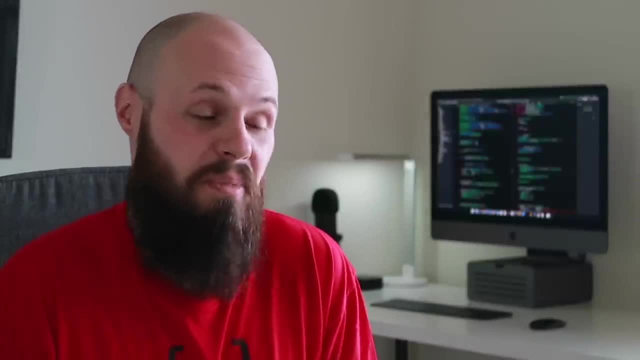 people offer that i don't know who, but just find somebody who earlier in your career can help guide in and get you over those hurdles. i know, when i first started out i didn't really have this for the first year of my career and when i got stuck i'd be stuck for days, and it was not only did it. 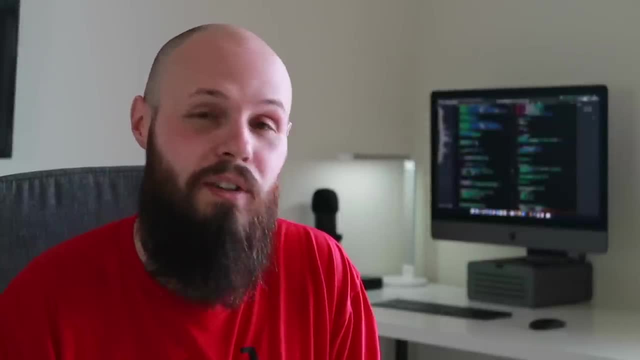 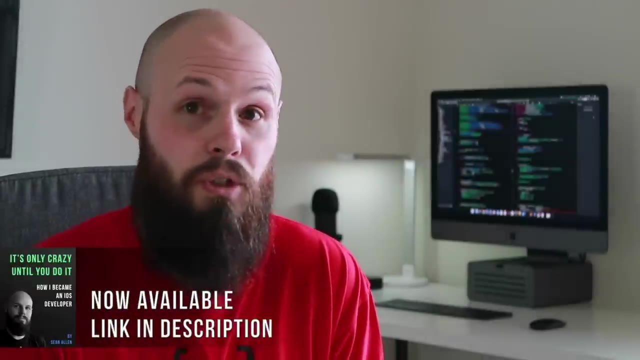 like slow me down, but it was discouraging, right? nobody likes to be stuck for days on a simple problem, when you can reach out to a mentor and just say, hey, can you explain closures to me real quick? i say that because closures hang up a lot of people and then having somebody- a mentor- explain 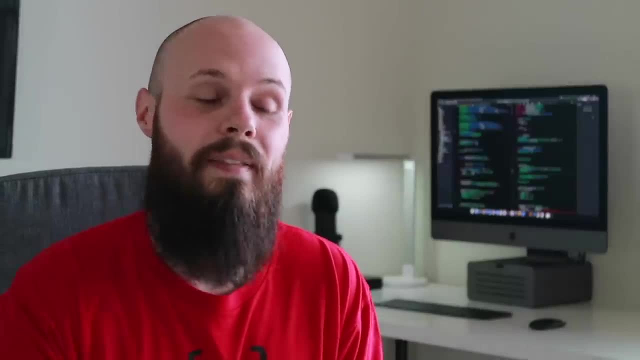 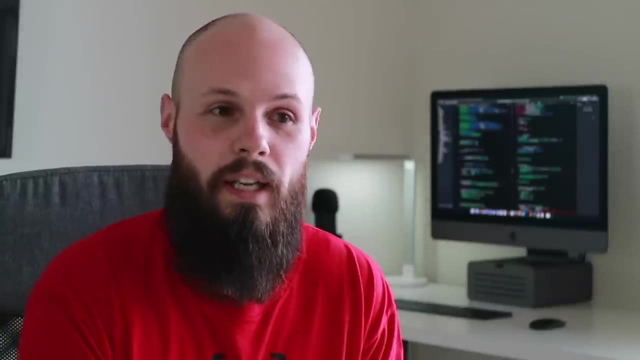 that to you can help get you over that hurdle and back on your way again. that'll speed you up and you'll be able to get it back on the road to making sure that you're not stuck on it. so if you're not stuck on that road, don't spend less time being discouraged, which the more time you. 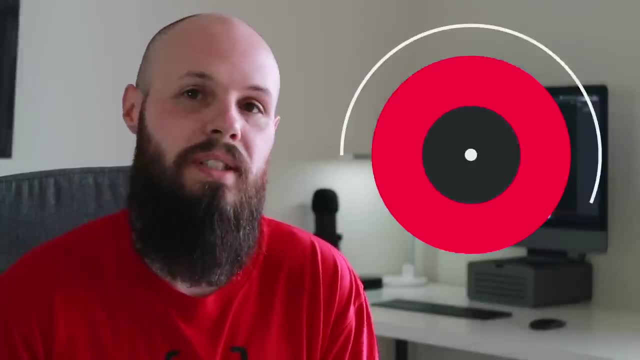 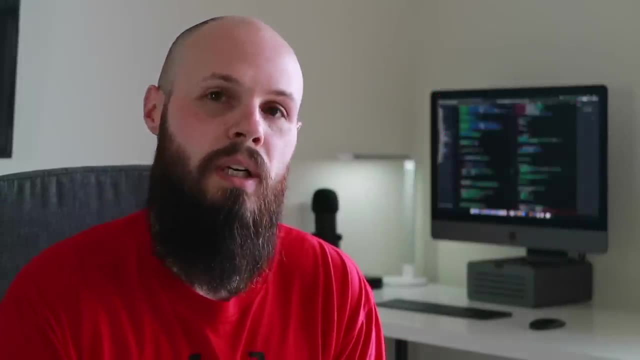 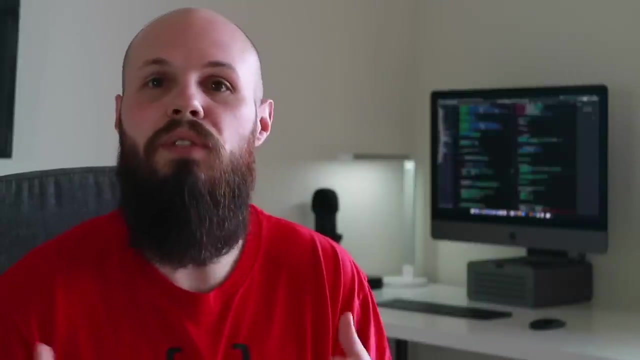 spend being discouraged, the more likely you are to quit and not complete this journey of becoming a software developer. my next piece of advice is i would start diving into the documentation of not only your language but the platform whichever you're working on- you know, ios, web, android, whatever- as soon as possible, kind of like i said before many of us start off doing tutorials. 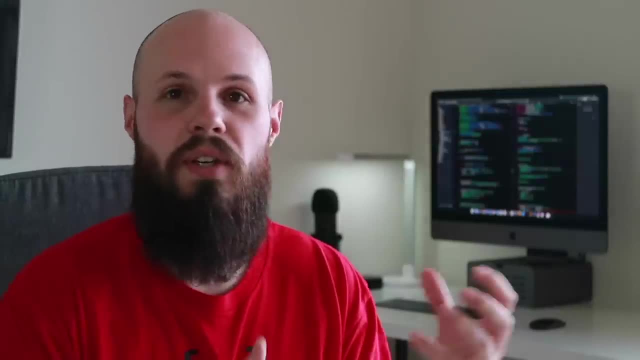 and that's how we start learning. but, like i said, once you can be self-sufficient and not rely on a cookie cutter tutorial, you can say: hey, i want to build a network, i want to build a network, i want to to build this certain aspect. and then you go to the documentation around. you know that aspect of 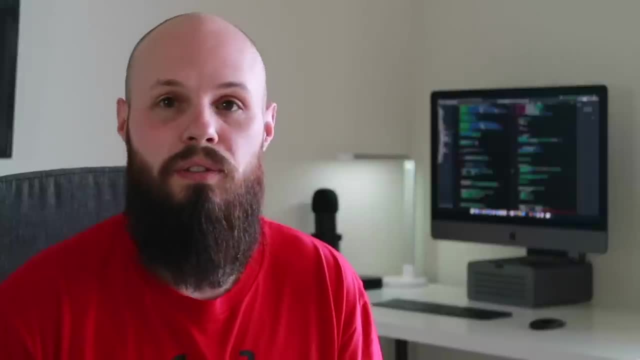 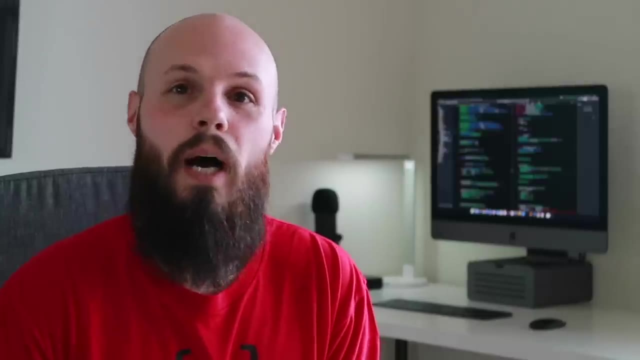 the platform, you can dig in and you can figure it out for your own. now you're self-sufficient and- and that's how you really get things done, that's how you get out of that tutorial trap that I mentioned earlier. and now you're on your own, building your own ideas, and you're on your way. 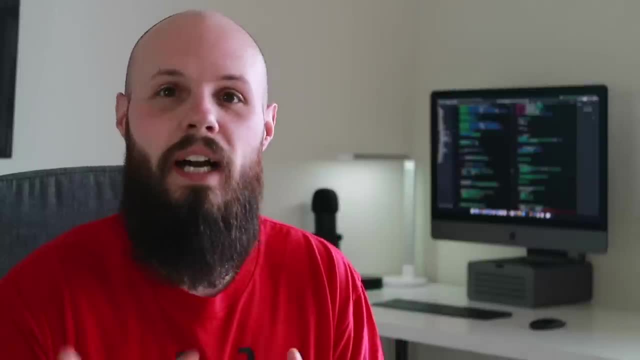 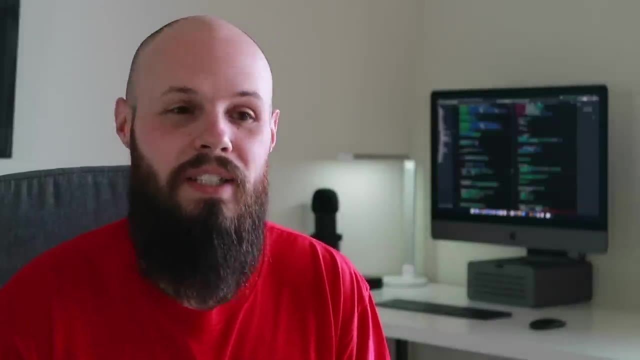 so the documentation, I know, can be a little daunting, especially in the iOS Swift world. it's not exactly straightforward and I get tons of requests for hey, can you do a video on how to read the documentation. but I thought about how I would do this, but truthfully, it's one of those. 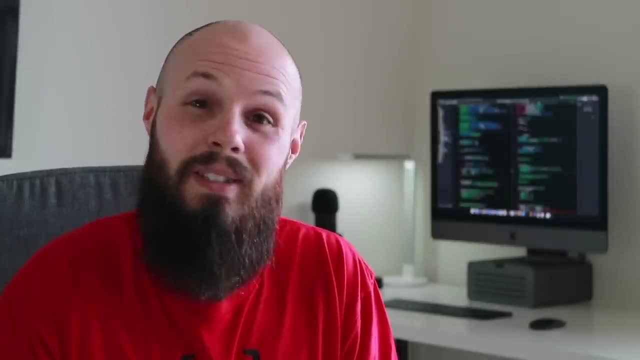 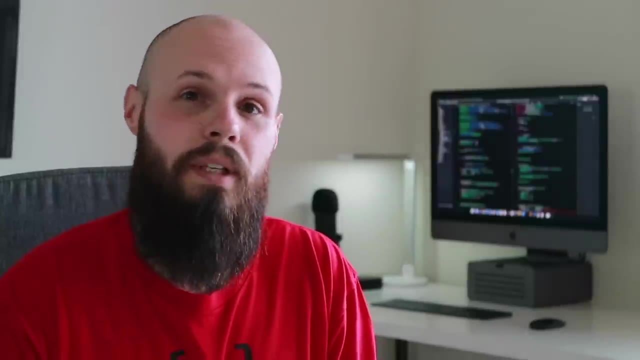 things where you just got to dive in and it it sucks, but it just gets better and easier over time. you kind of got to go through that learning curve, so fortunately there's no magic bullet here. but just dive in as soon as possible and you'll get through that rough patch and be out the other. 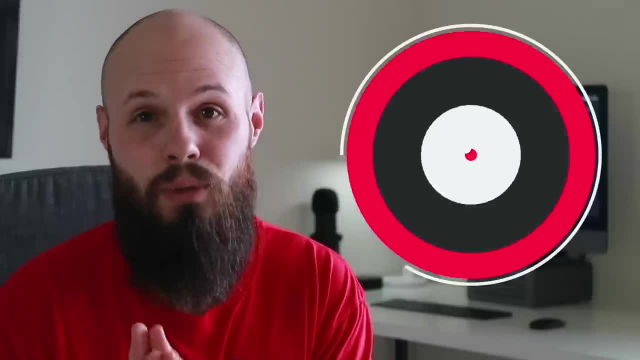 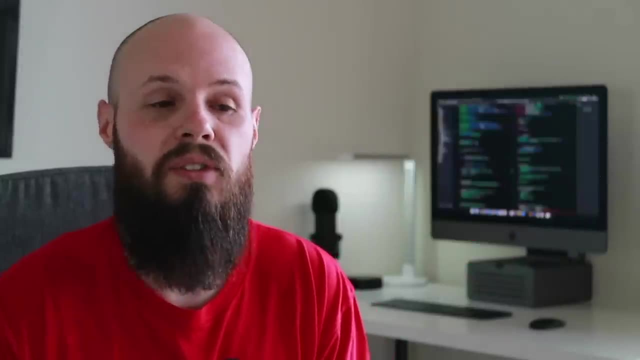 side faster than you know it. the next advice is that you have to love it. luckily, I do love it, but I I talk to a lot of beginner programmers who are inexperienced or just getting started and truthfully they do it for the money right. we all know software developers get paid pretty well. 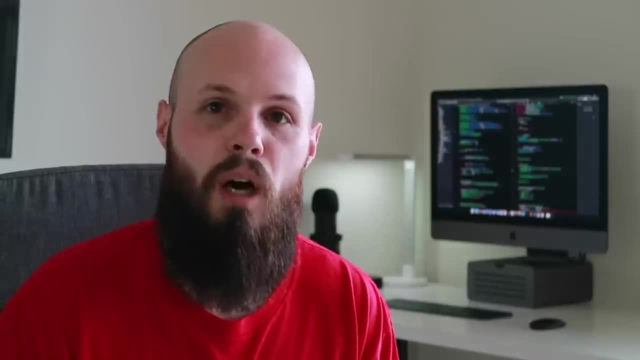 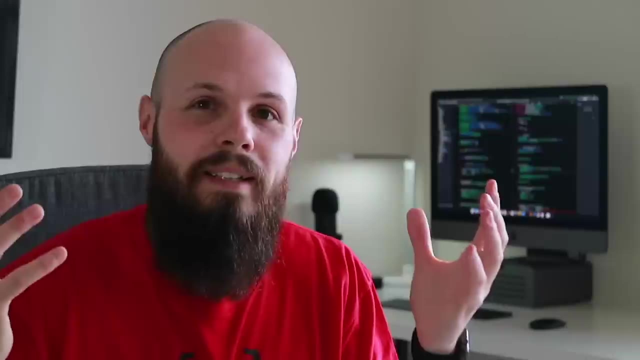 and that's the only reason they do it. they don't do it because they love to solve problems, or they don't do it because they love to build or create things right. that's the reason you should be doing it is because you- just you- love the fact that you can take an idea in your head, type on a keyboard. 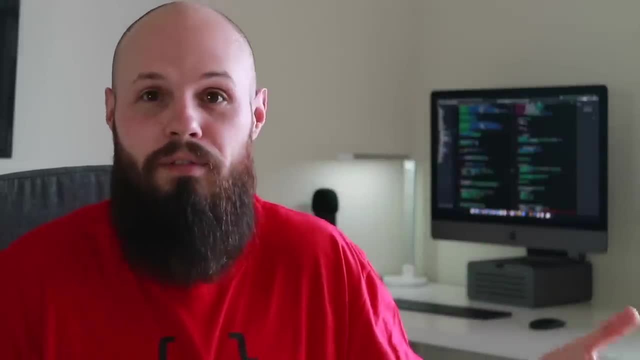 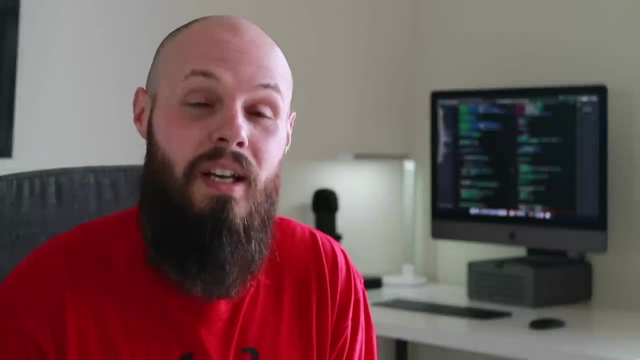 with those colored text back there and then something magical pops up on a phone, like if that is just so enticing to you, you're in it for the right reasons and, again, you just have to love this because, kind of like I mentioned earlier, you're going to have to love this because you're 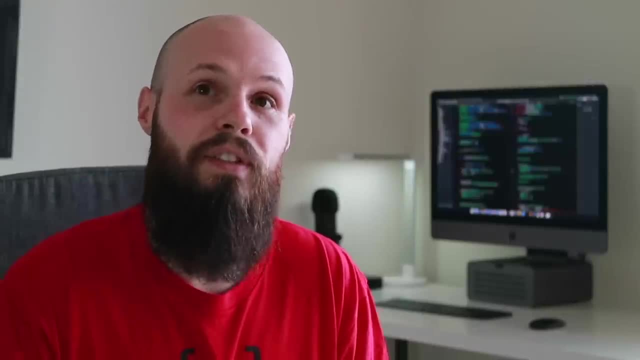 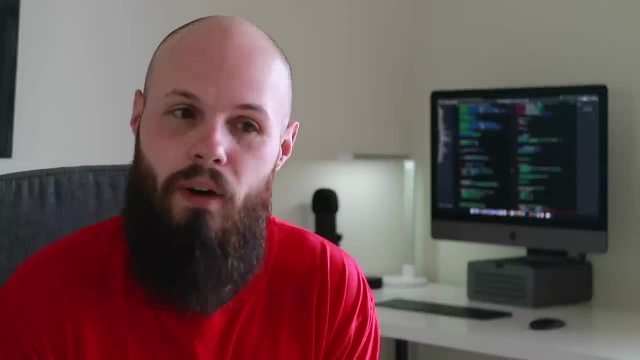 going to run into rough patches, you're going to hit roadblocks and if you don't love it, those roadblocks are gonna knock you down and you're probably gonna give up. however, if you love it, you're gonna kind of take those challenges head-on, plow through those roadblocks and be on your way. 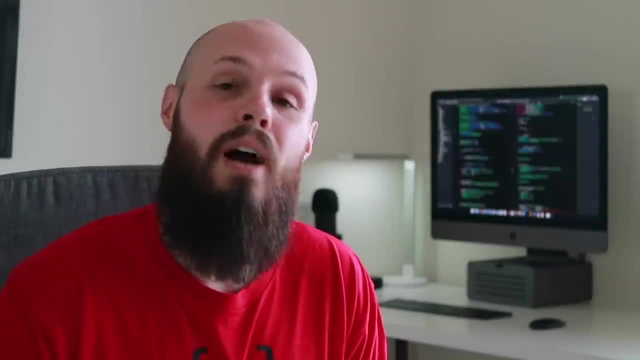 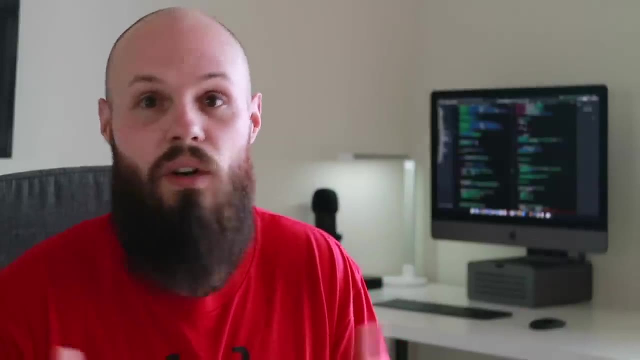 and newsflash. those roadblocks don't go away. doesn't matter how senior you are, how long you've been doing this. technology is always changing. something new is gonna come out- AR kit, AR glasses, VR, whatever- and you're gonna have to learn all over again. so if you don't love the process of 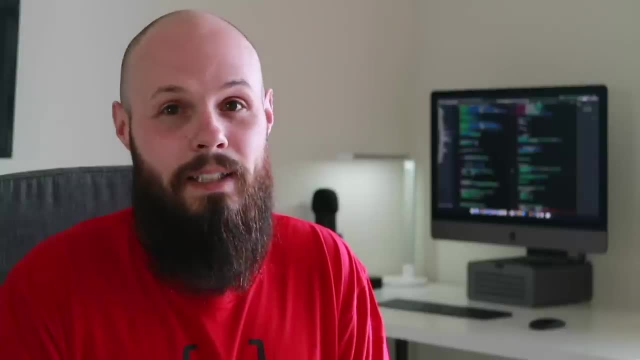 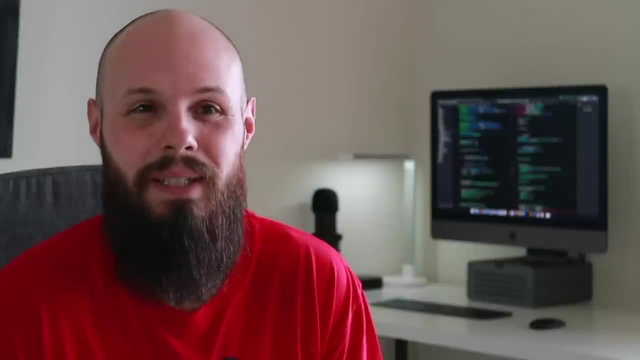 learning and solving problems, you're gonna have to learn all over again. so if you don't love the process of learning and solving problems and building and creating, it's gonna be a rough road. so, again, you have to love this. building on that, because I just kind of talked about how rough it can be. but it does get easier and here's why. 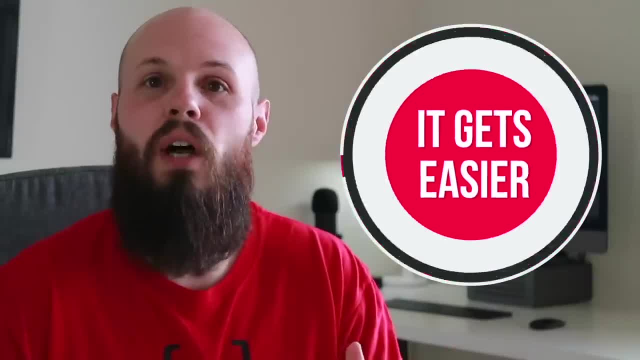 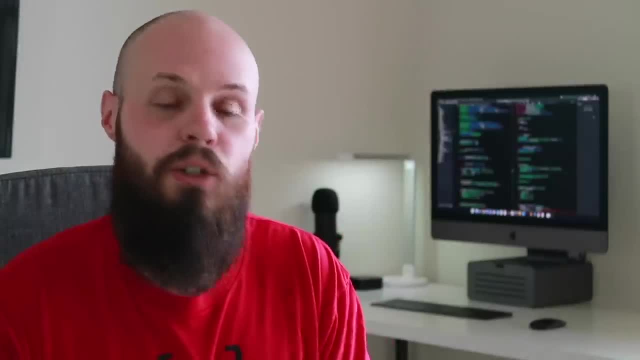 as you go through your career like it's gonna seem super daunting that you know there's all these possibilities of apps you can build. however, as you go through your career, where there's contracting, working in other companies, you're going to be building various different apps and 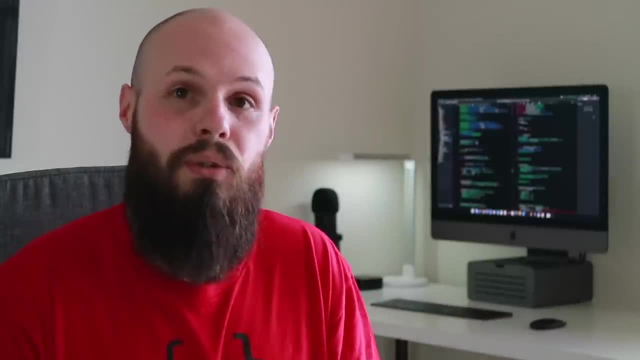 when you build these apps, you're going to have these code bases on your hard drive, so you'll have access to previous code bases and you'll have access to different code bases, and then you have access to previous code bases, and then you have access to previous code bases, and then you can. 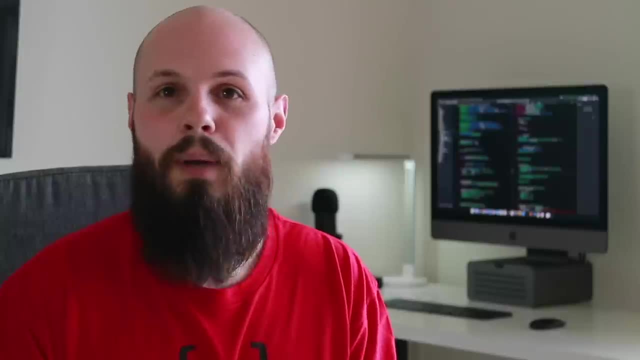 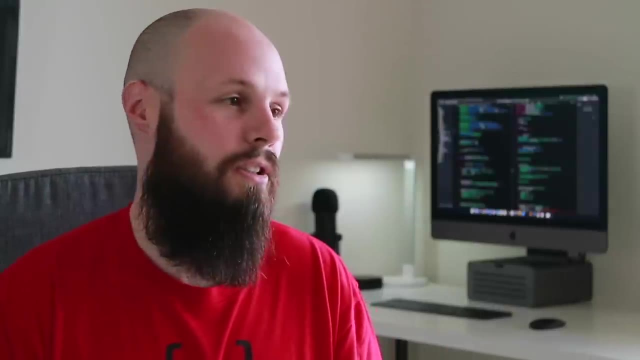 code you've written to use in future projects. Now I'm not saying you're just going to copy and paste that code. but let's say you built a fully fleshed out custom camera screen and then two years later you're going to. 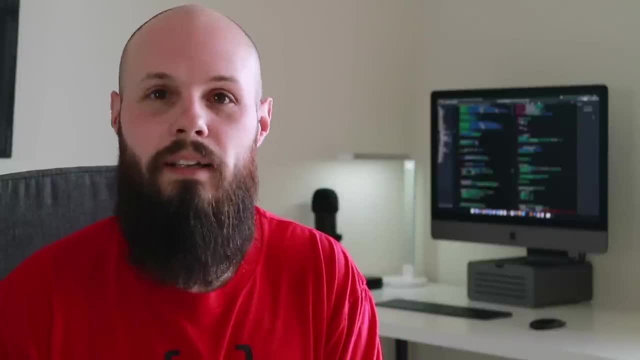 build another camera app and you're like: oh, I've done that before, Let me go back And again, you're not going to copy and paste it, but you're going to have a lot of the heavy lifting has already been done for you. 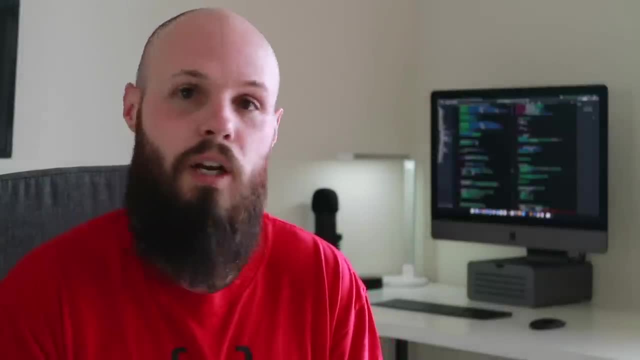 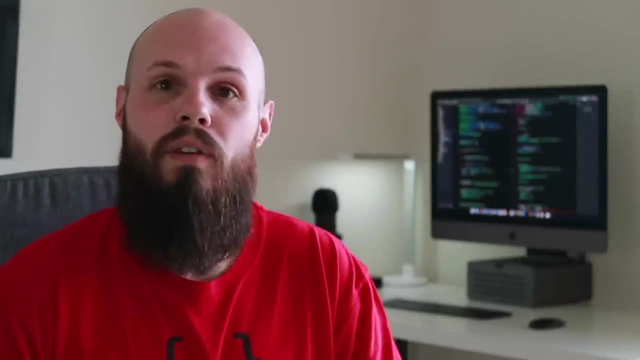 So what I've found? I've built probably now 10 production apps between contracting and startups. Over time I have built many, many features that can be done on an iPhone. So whenever I come across something tricky, I know that I can always go back to I call. 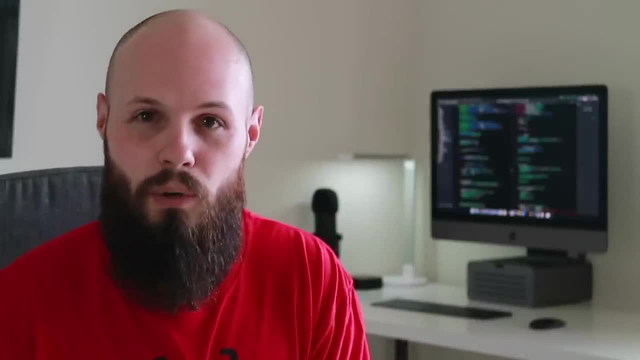 it my toolbox. I can always go back to my toolbox of code, see what I've done before and pull from there And again. a lot of times the heavy lifting has been done and I just got to tweak it or add some little stuff. 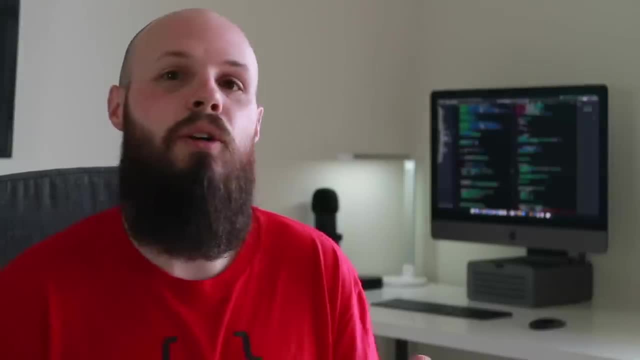 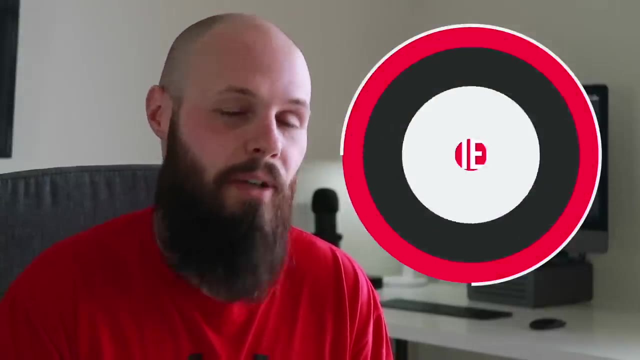 So it does get easier the longer you do it, And then, as always, I want to preach patience Again. so many people reach out to me and say: how can I become an iOS developer as fast as possible And right away? you already have the wrong mindset. 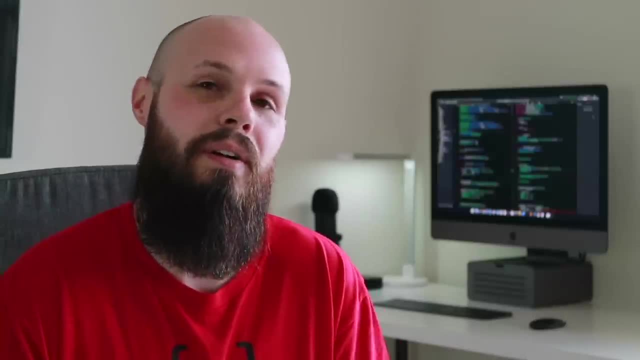 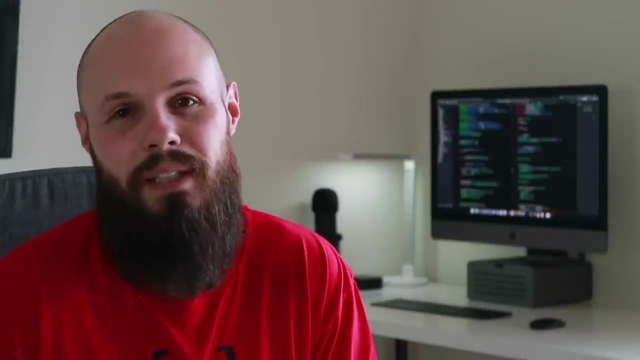 This is such a marathon. It's not a sprint. It is a very, very long journey And if you're just trying to get there as fast as possible, all the other stuff I talked about earlier in the video is really going to come and bite you in the ass. 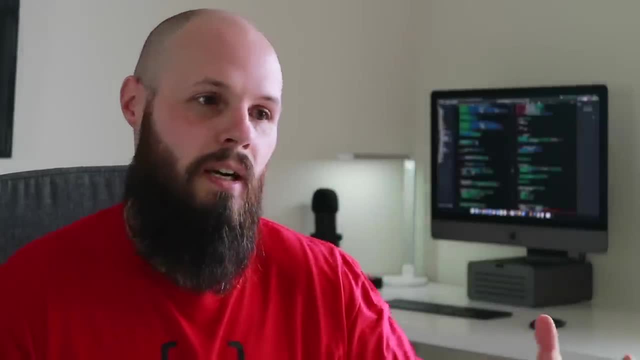 So just be patient And don't compare yourself to somebody else as well- Like this happens to me sometimes, right, I've been doing this for about four years And I look at developers who've been doing it for like eight and I'm like, oh man. 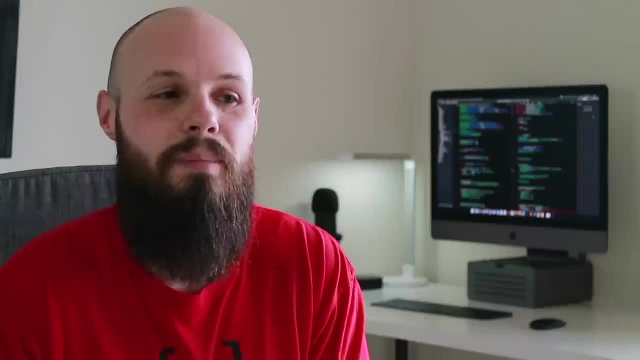 I'm not as good as them. It's like they've been doing it twice as long as you, So it's hard to compare yourself to other developers. You're on your own journey. It's going to take a while And, like I said before, if you love it, you're determined. 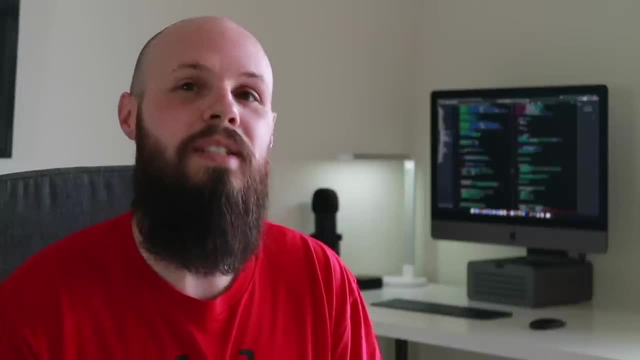 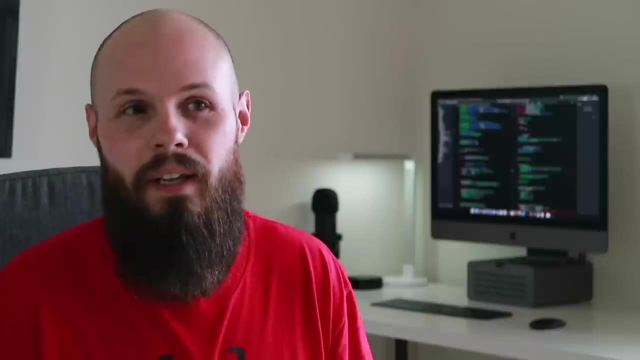 You're going to get there. Just keep plugging away. But just patience is the key. If software development was so easy that you could learn it in two months, everybody would be doing it. The market would be oversaturated and it wouldn't be such a coveted position. 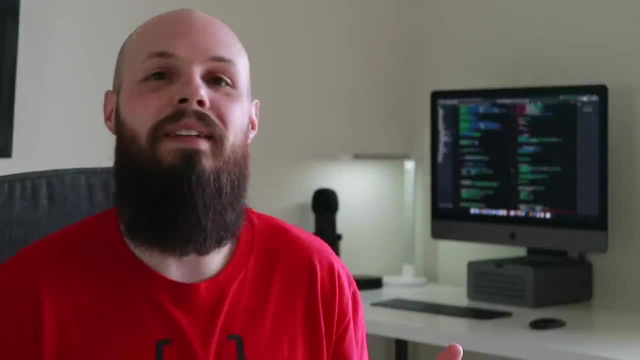 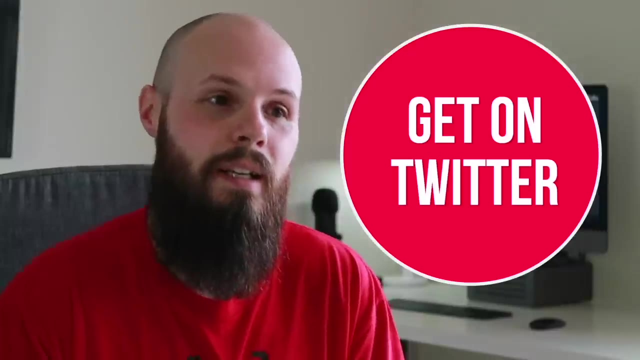 So have patience, It'll pay off in the long run. And then, finally, probably my most important piece of advice- I've said this time and time again- Get involved in Twitter ASAP. It took me two years to finally start interacting in iOS conversations on Twitter. 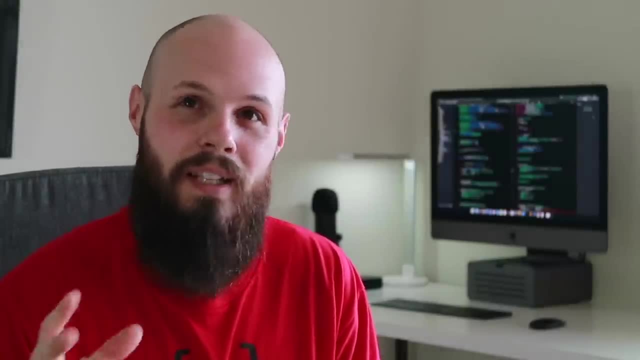 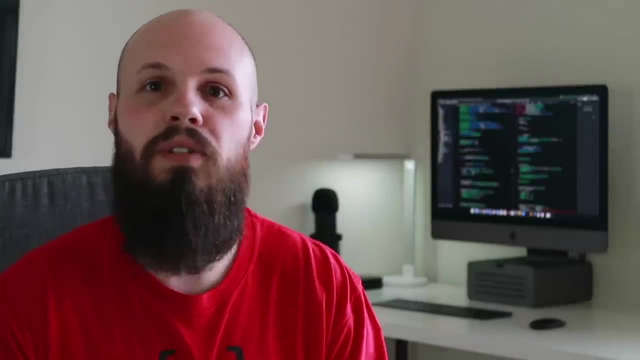 And I just kick Myself all the time. This sounds like a bold statement, but I would say Twitter is the most important tool for my developer career. Just the people I've met, the developers at other companies I've, you know, gotten to know and meet, you know, through Twitter. 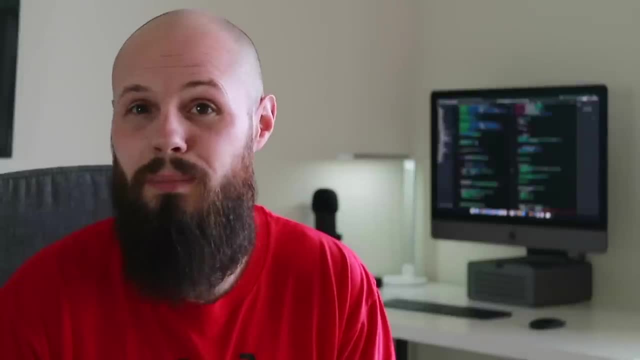 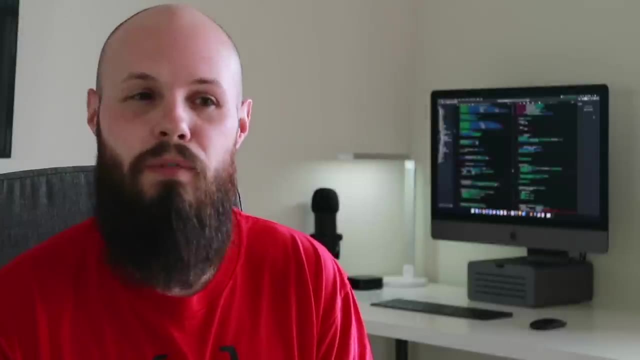 It's amazing- And I can really only speak for the Swift community, but the iOS and Swift community is amazing on Twitter: Super helpful. I know Twitter may have a bad rap for some of you, but Twitter has like a lot of different types right. 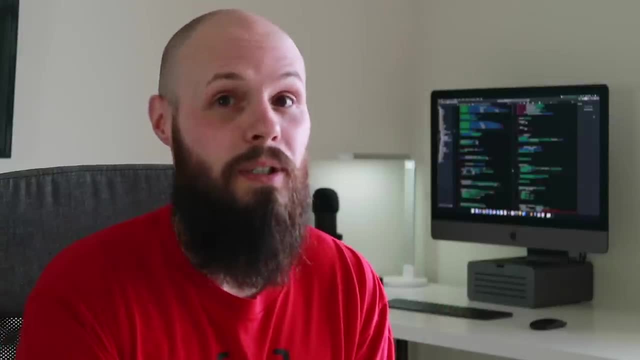 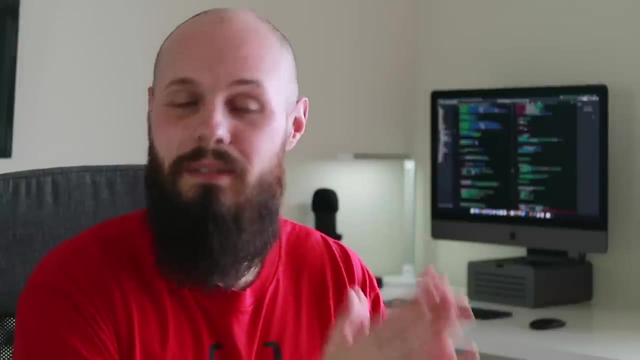 Like there's sports Twitter, financial Twitter, Software developer Twitter, at least in the Swift world, is amazing. Obviously like political Twitter is probably a cesspool, but you know, developer Twitter great. This is a big part of how networking is done in the software developer world. 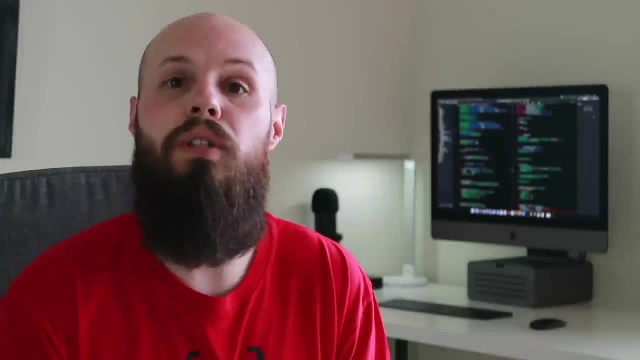 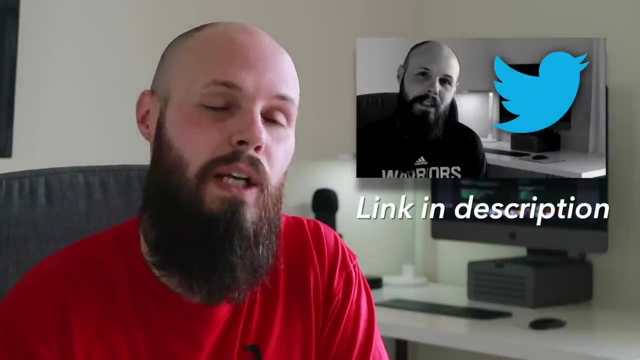 You interact on Twitter. Next thing, you know you meet somebody at a conference and they know you because you've been interacting on Twitter. It's anyway. I could go on for days and I did in this video, Check it out, But Twitter is so valuable for a developer. 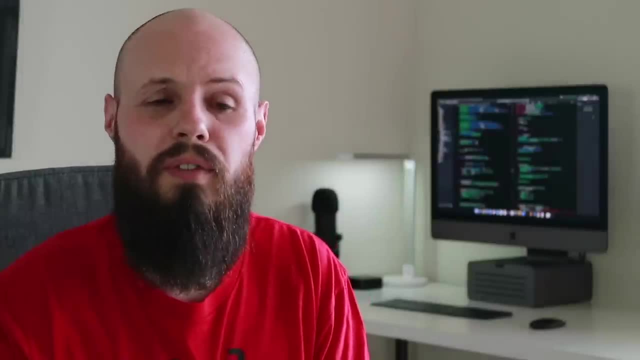 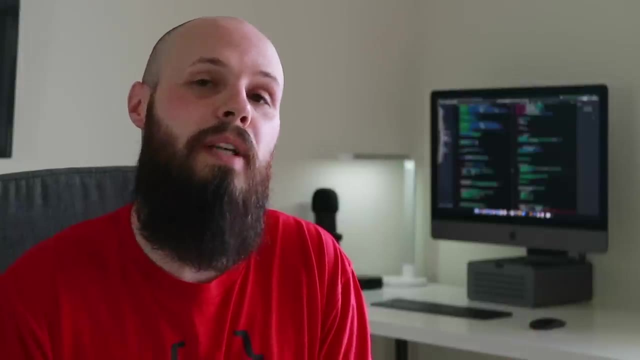 And I again. I wasted two years being scared to jump into a conversation. Don't do that. Start. Start right away, and you'll be happy you did So. those are the nine things I wish I knew before I became a software developer. 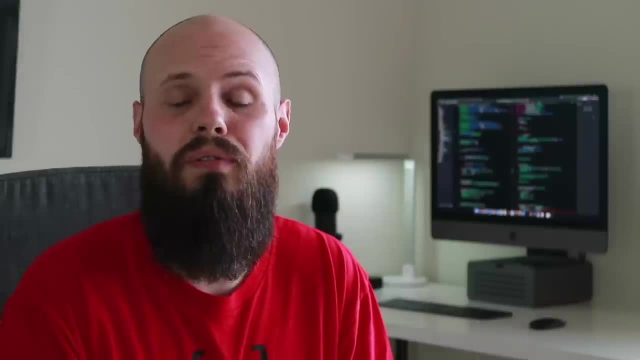 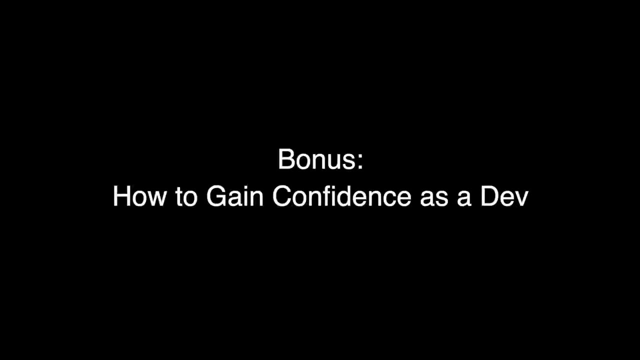 I hope some of that helped you out. If you like what I'm doing here, I put out a show called Swift News every Monday in a tutorial or two throughout the week. We'll see in the next video. What's up everybody. 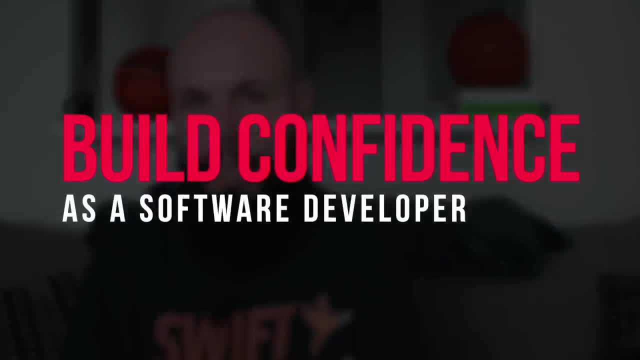 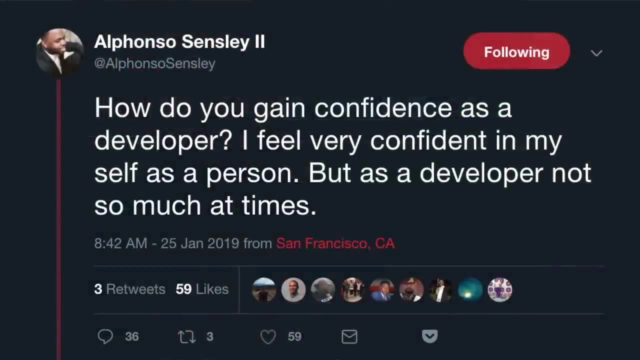 Today's video is going to be all about building your confidence as a software developer. Now, we've all heard of imposter syndrome. We probably all experienced imposter syndrome, But this video really stems from this tweet here from Alfonso. It says: how do you gain confidence as a developer? 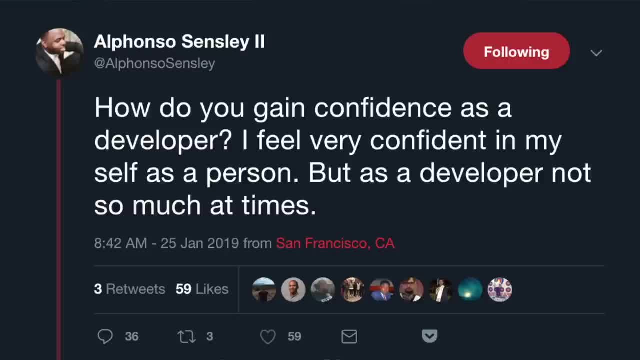 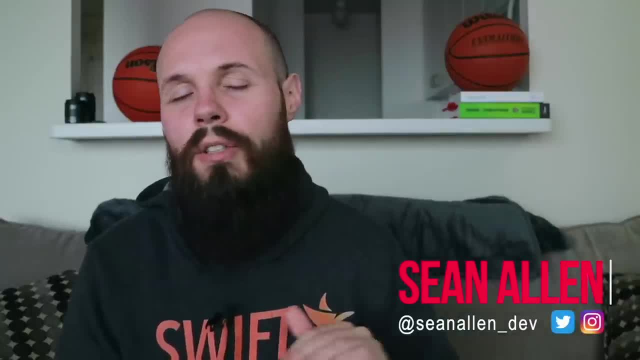 I feel very confident in myself as a person, but as a developer not so much at times, And I'm going to link to this tweet. in the description There's like 40 something responses to this thread- Great stuff. I picked out a few of the responses and I want to talk about some of these topics on. 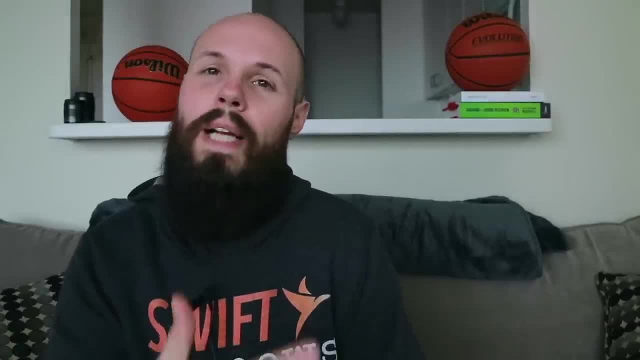 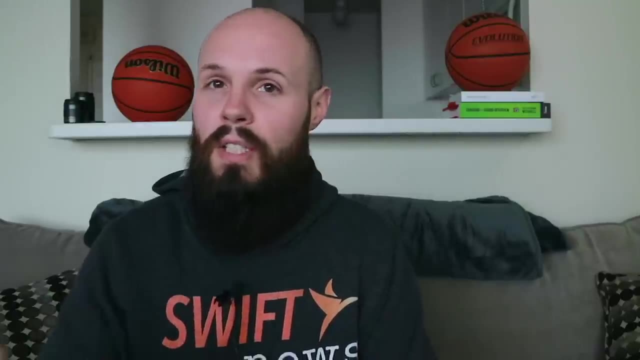 how to build your confidence. Just to give some quick context on Alfonso here: I've been interacting with him on Twitter and in the YouTube comments for well over a year now. I've actually met him at a startup He's been working on becoming a self-taught iOS developer. 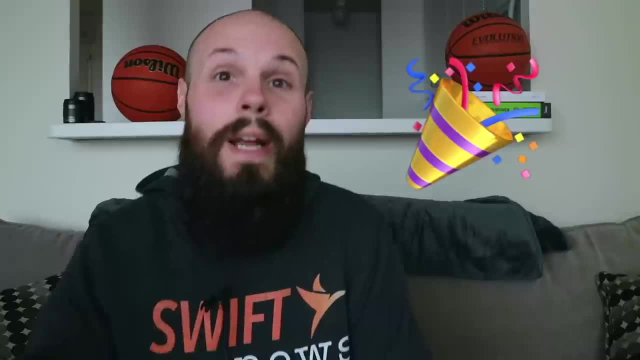 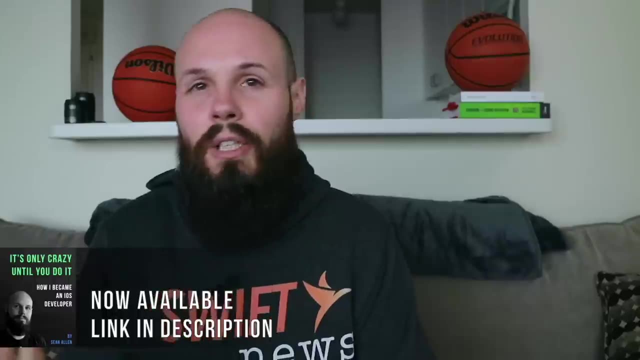 For a long time now and recently just got his first job. So, hooray, Congratulations, Alfonso. But that's the context around this tweet. He's just now starting his first job and the confidence is shaken a little bit Now. the first two responses I want to touch on are from Zach and Corey. 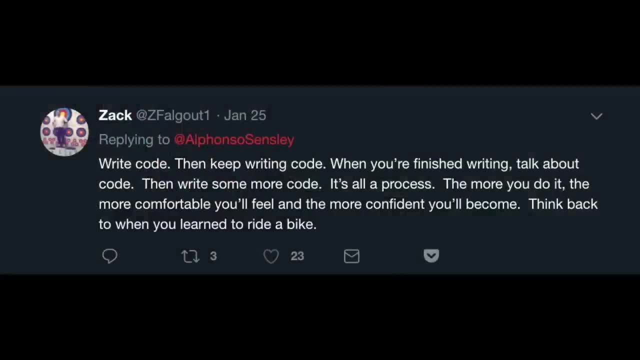 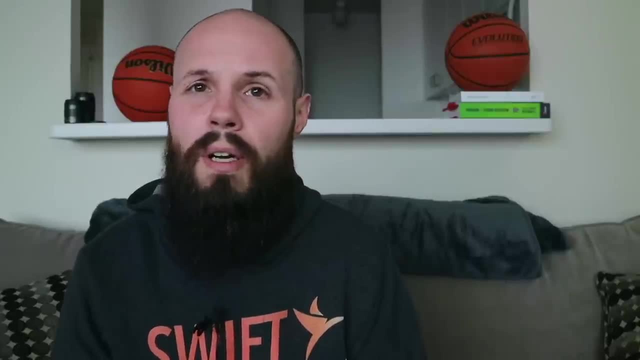 And Zach says: write code, then keep writing code. When you're finished writing, talk about code, then write some more code. It's all a process, The more you do it, et cetera. And the point Zach touches on that I want to elaborate on is just this concept of immersion. 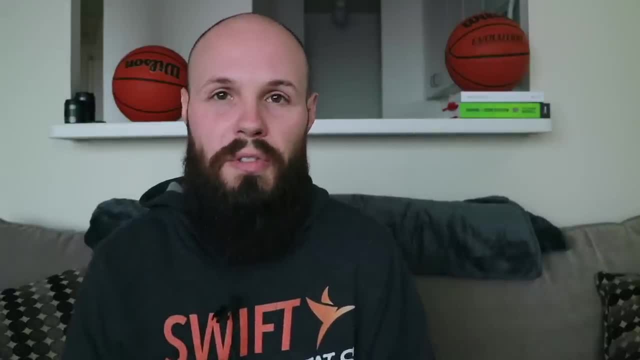 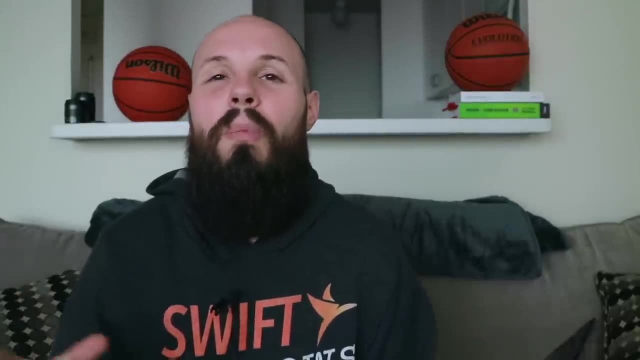 with people like learning, development, just completely immerse yourself and soak up as much knowledge as you can, whether that's YouTube videos, books, podcasts, blogs, like just completely immerse yourself in this world, And the more you do that just over time, like knowledge is power. 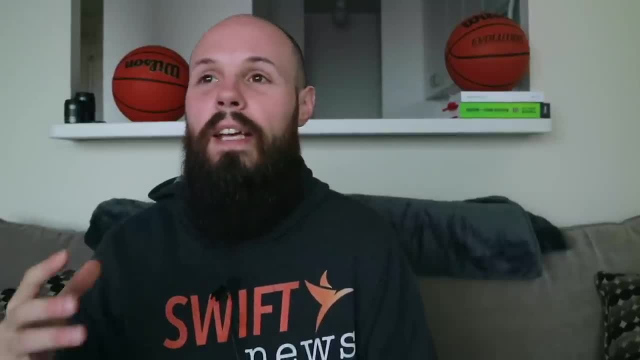 You're just going to increase your knowledge just day by day, by day by day And just over time, like the more you know, the more confident you'll become. And then Corey says: you know? for me it's looking back at how I didn't know a single. 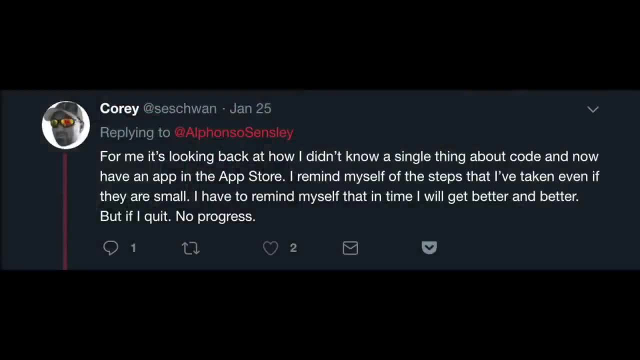 thing about code and now have an app in the app store, I remind myself of the steps I've taken, Even if they are small, you know. I have to remind myself that in time I will get better and better, But if I quit, no progress. 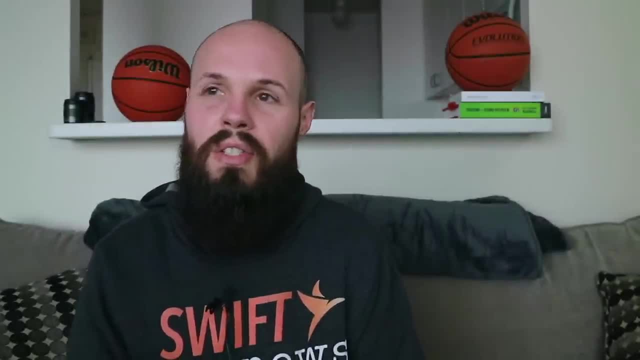 And that builds on what Zach says, and what I want to touch on is just the concept of patience. Yes, I mentioned immersion a little bit ago, but you can't just immerse yourself in three days later Be confident in all your knowledge, right? 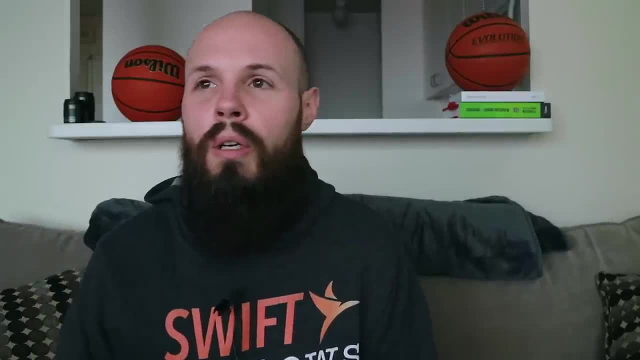 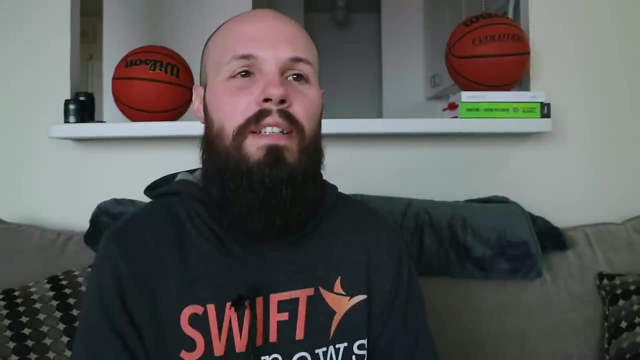 It's going to take time. So just knowing in the back of your head that this is a long, multi, multi-year journey that might not give you the confidence but that will help you deal with that feeling of lack of confidence. Know that everybody started out. you know as a beginner. 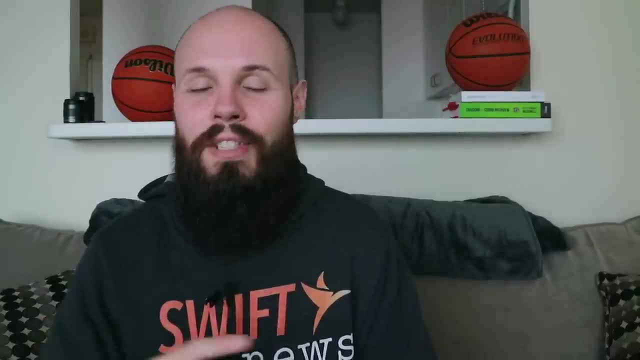 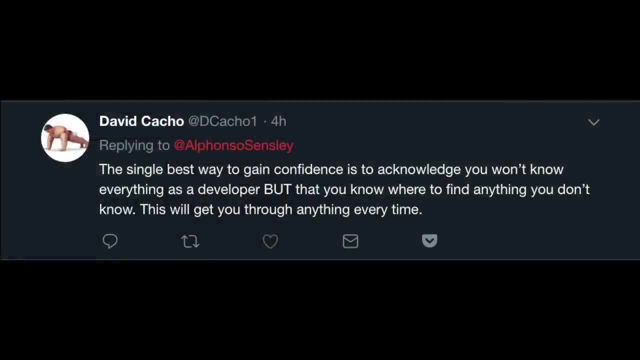 As a beginner at one point. So just know that this is your journey is going to take time. The next response here from David Cacho. it might be my favorite one because I think it resonates with me the most- And it says the single best way to gain confidence is to acknowledge you won't know everything. 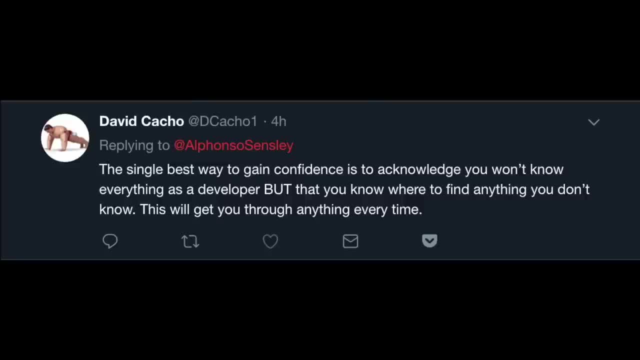 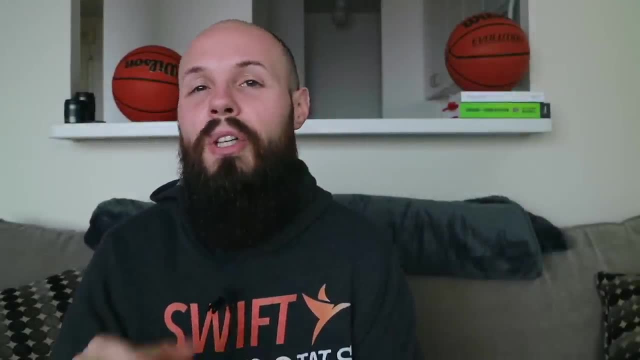 as a developer, but that you know where to find anything you don't know. This will you get. this will get you through anything. every time, And I always say: the biggest thing as a developer is: you need to learn how to learn right. 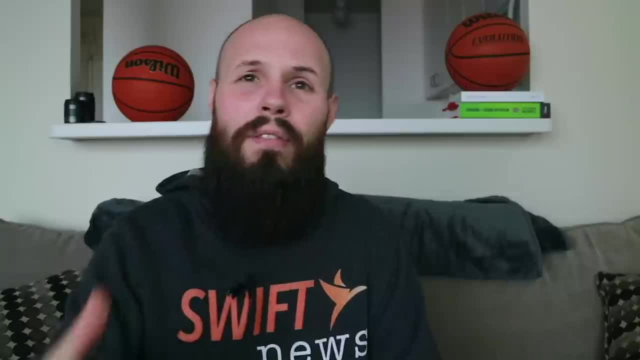 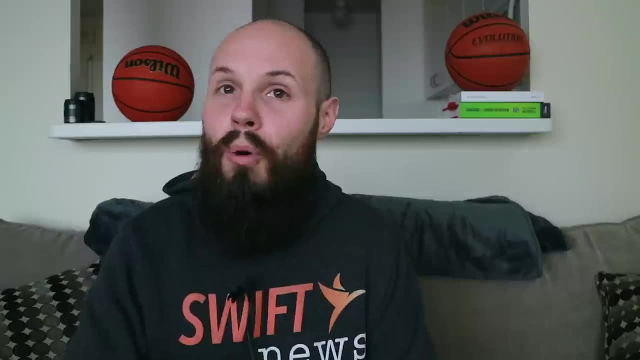 Because- because, like David says, it's impossible to know everything about every developer, Every development language or every you know framework within that language, etc. You just can't know that stuff. But if you know how to learn, that will boost your confidence because, like I know, that's. 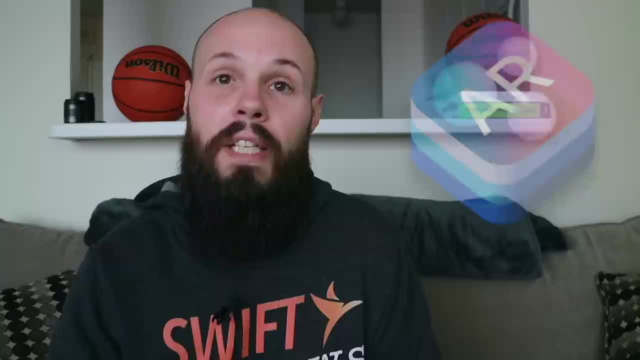 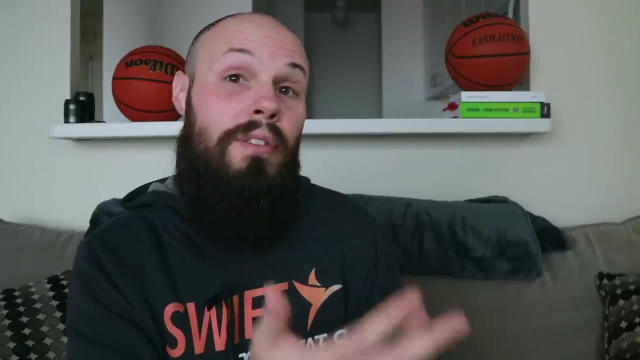 kind of where I'm at is, say, I go to a company that works with ARKit and they're building an augmented reality app. I've never built an ARKit app but I'm not worried about that because I know that I will again back to the first. you know responses. I would completely immerse myself, you know. 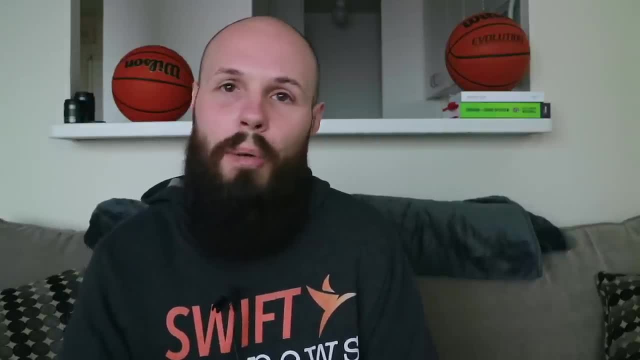 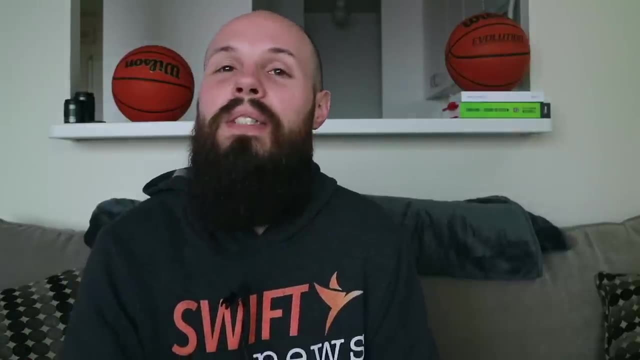 and, given you know, a few weeks in time, I'll be caught up to speed and I'll be good to go. And the reason I have confidence there is because I know how to learn things like right, Like I'm confident in myself that I will pick it up quickly. 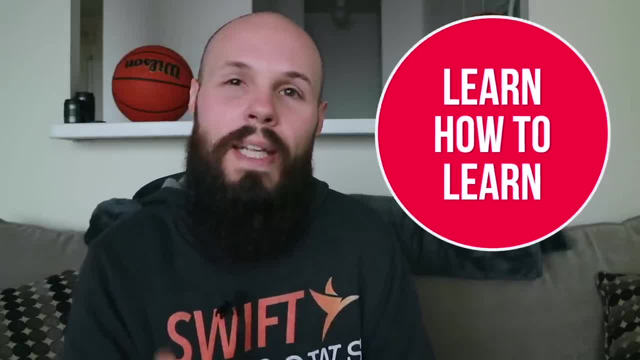 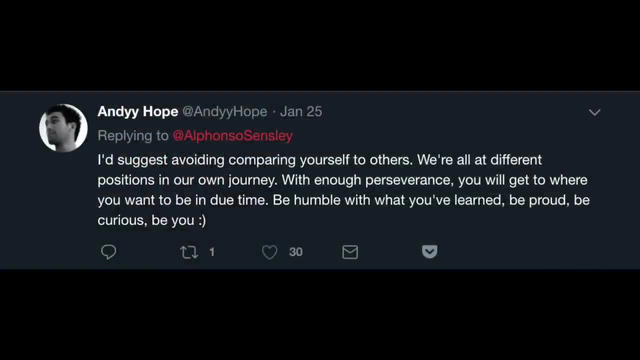 So again, I will work on that skill. if you want to build your confidence, Learning how to learn might be the most important skill as a developer. Next up we have a good one from Andy Hope that says I suggest avoiding comparing yourself to others. 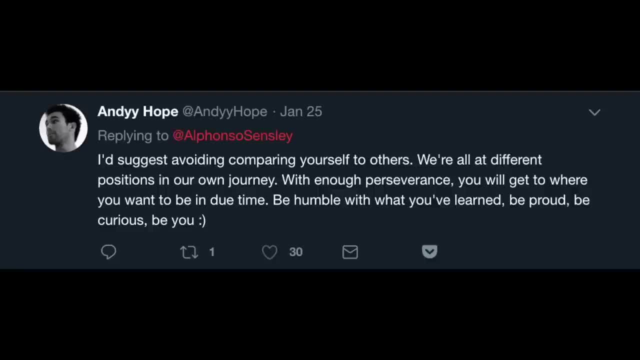 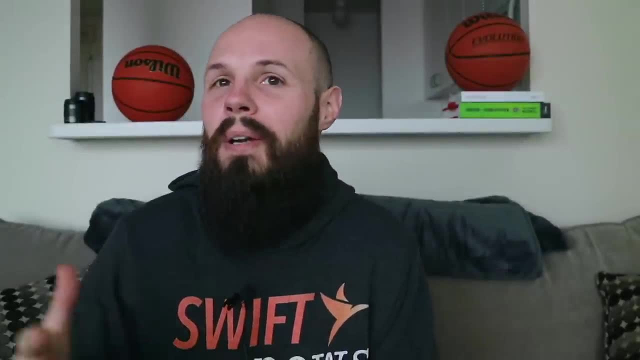 We're all at different positions in our journey. With enough perseverance, you will get to where you want to be in due time. Be humble with what you've learned, Be proud and be curious and be you. So the message here is: Just don't compare yourselves to others, like you're on your own path. 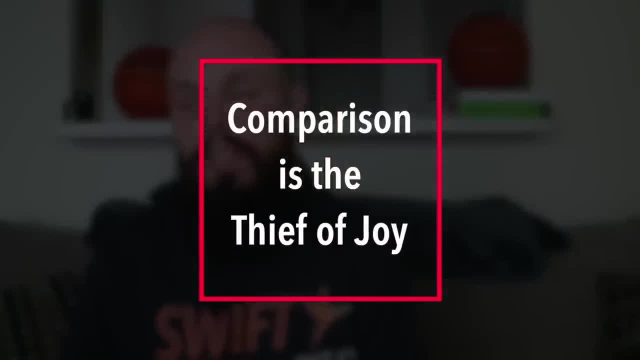 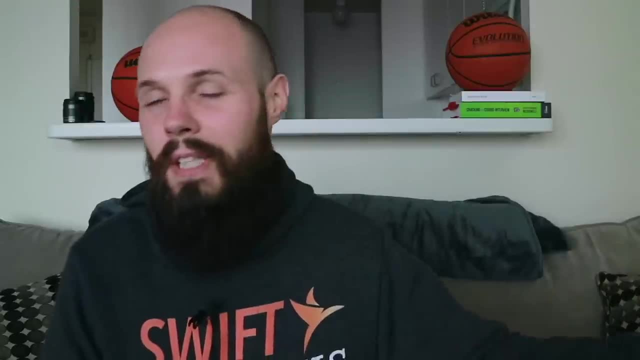 There's a nice saying that I love. It's called: comparison is the thief of joy. Just do you be you. be on your own path and don't worry about like, oh, this person knows more than I do, Like you don't know their history. 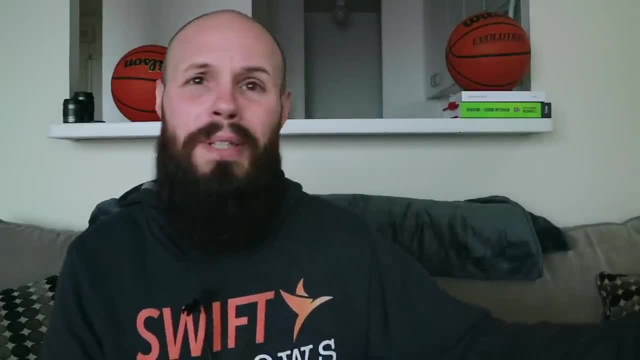 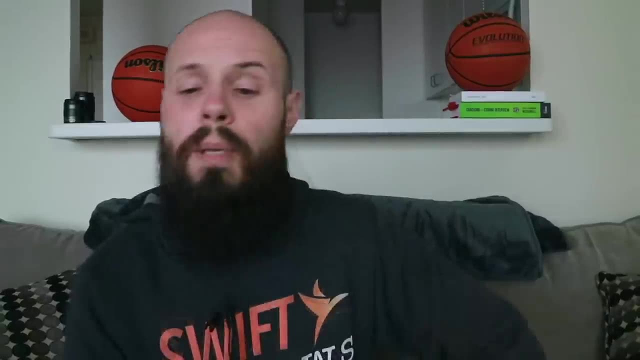 You may be self-taught. You wrote your first line of code three years ago. They may have been coding since they were 12, right? That's not a fair comparison, So don't compare yourself to other people. You're on your own journey. 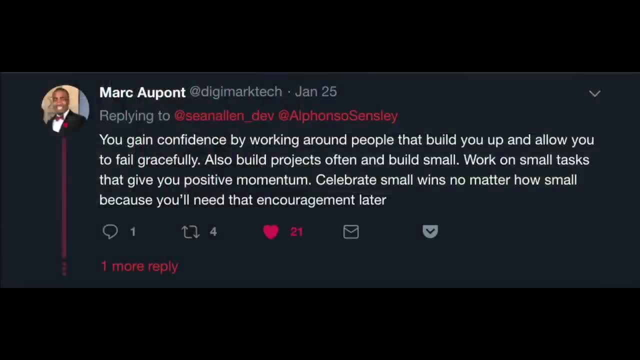 Next up I want to talk about Mark Oppont's response. A little fun fact about Mark: He was the first ever guest on Oracle Origin stories. My podcast Got to get the plug in, you know. But anyway, Mark says you gain confidence by working around people that build you up. 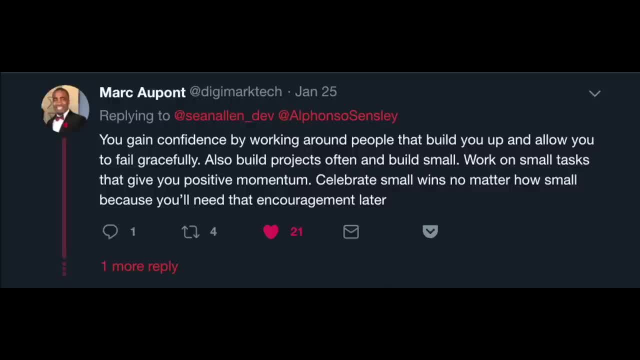 and allow you to fail gracefully. Also, build projects and build small work on small tasks, et cetera. Really, really, what I wanted to focus on with Mark's response is, you know, gaining confidence by working around people that build you up and allow you to fail gracefully. 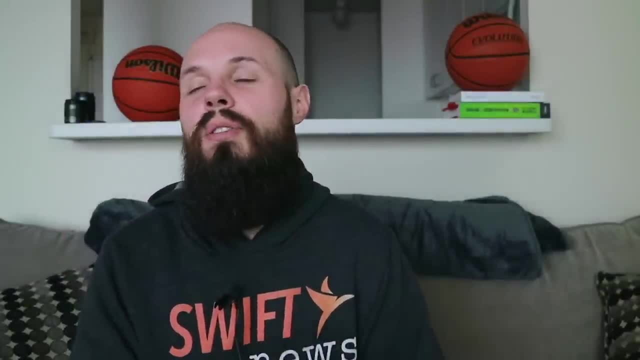 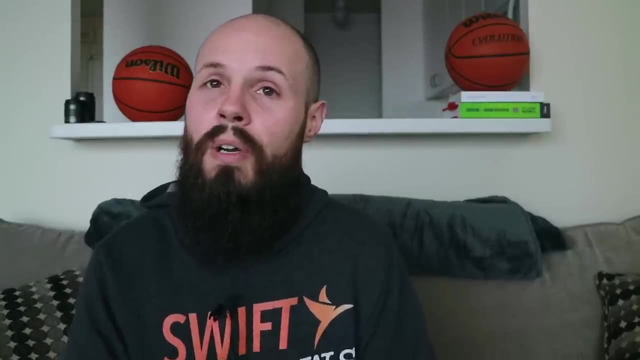 Because really what I want to elaborate on is your environment is so so, so important right? Don't get me wrong. I know oftentimes if you're trying to get that first job, you may not have a lot of choices on where you go. 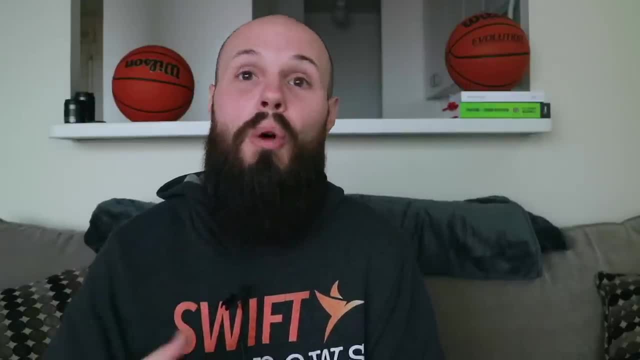 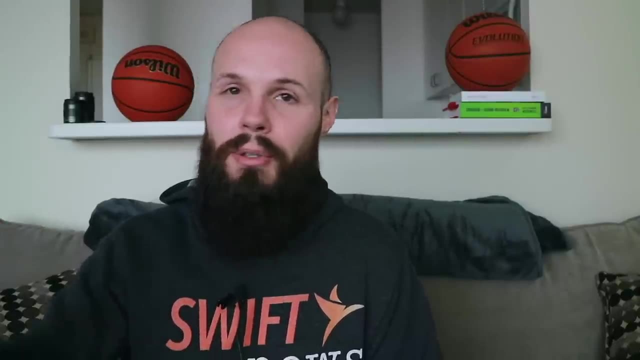 But if you are fortunate enough to have any choice, my opinion is to always judge the quality of team first. Like a lot, of people go for the biggest salary, and to me salary is like third or fourth on the list of importance and team is number one. 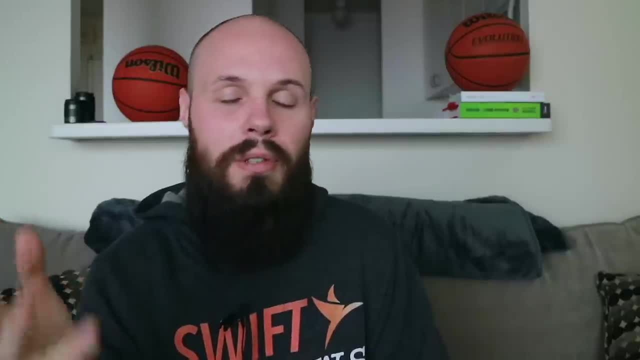 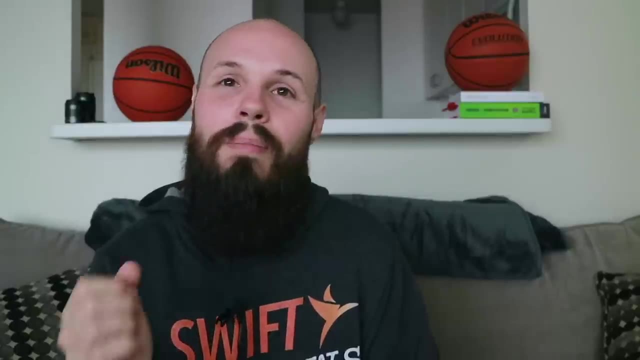 Think about it: You work with these people every day, eight, nine, 10 hours. however long you work, whatever, You spend more time with them than you do your family. So your environment that you build is going to have a major effect on your confidence. 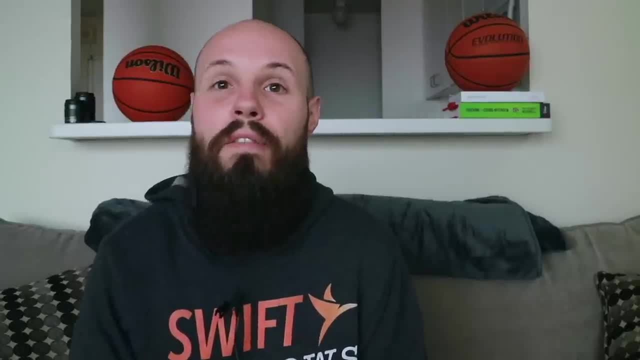 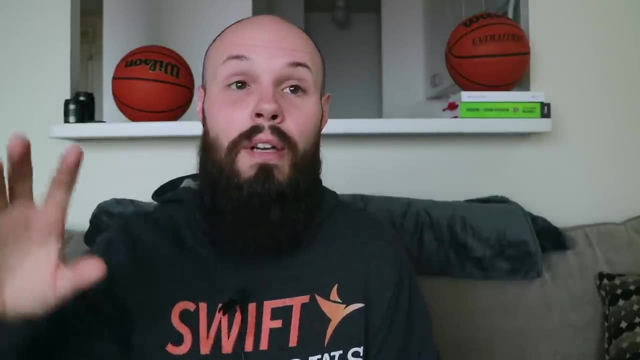 your career And just that vital, you know, first year of your career, Yeah, Having a good team that really boosts you up and good mentors, that can just shoot you off exponentially on an amazing career. Vice versa, if you're in a very, very toxic environment, that can just really depress. 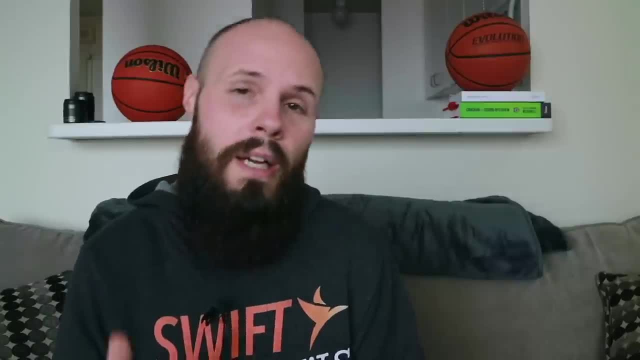 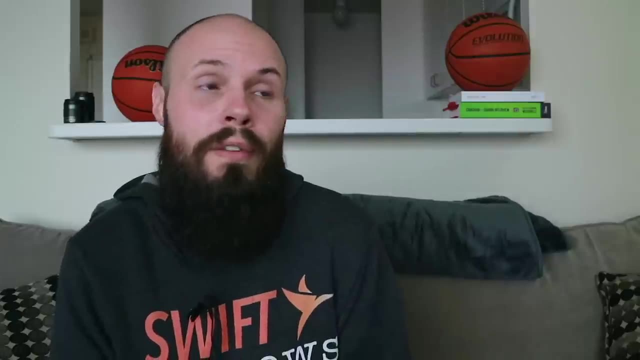 you and put you down and can really affect the whole rest of your career. So again I want to stress what Mark is saying here is: your environment is super important and that can really help with your confidence. Or even if you are a confident person and you go into a toxic environment, that can. 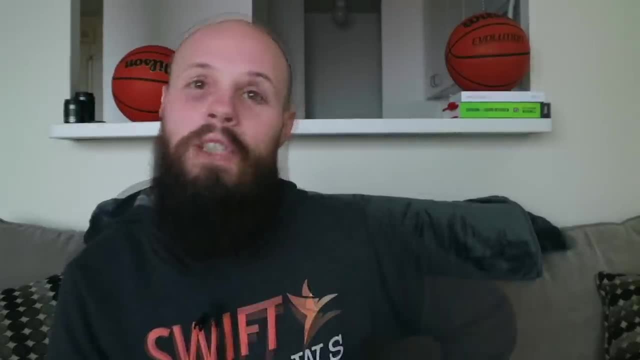 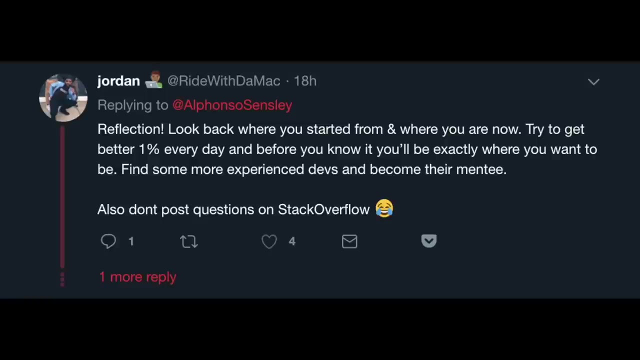 like: remove your confidence, So pay attention to your environment. Next up, we got a good response from Jordan here. It says: reflection, look back on where you started and where you are now. Like: try to get 1% better every day. 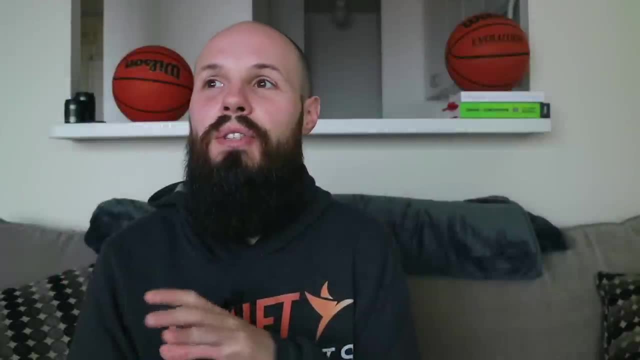 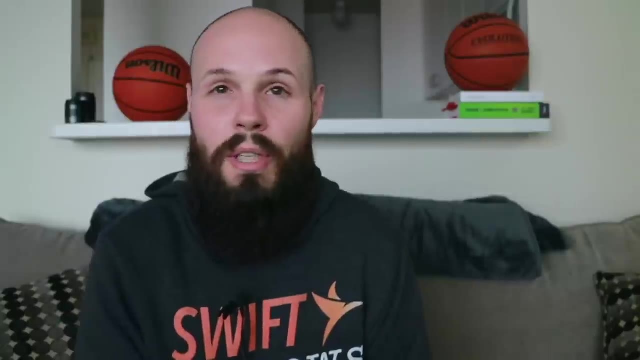 That's a very, very common saying, But basically what he says is just have context and perspective on how far you've actually come Like. this really resonates with me because I was a self-taught developer. you know, four years ago you did a bootcamp and you had been on my way, but it's just like you know. 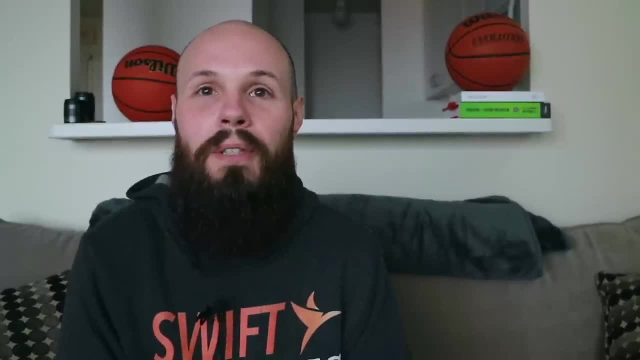 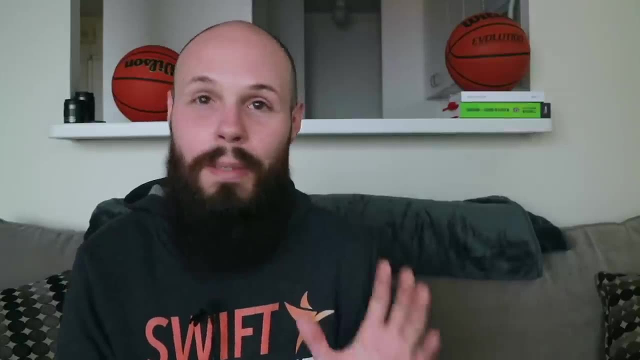 anytime I was lacking confidence. it's like man, you didn't even know how to code four years ago, Like now: look where you're at. It's just And perspective how far you've actually come and be like: yeah, I got this. 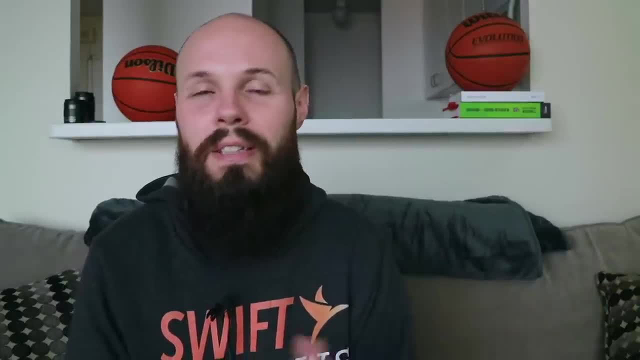 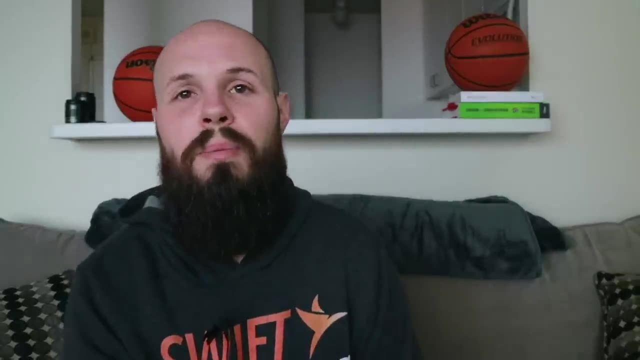 And then you know this is all building on previous answers- You're on your own journey, Like, don't compare yourself to others, Like and just again, perspective is the big key here. You've come a long way And the next comment I want to talk about is from Skye Brown and she says: I think building 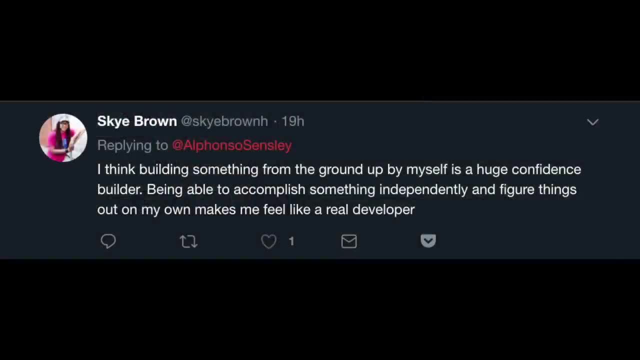 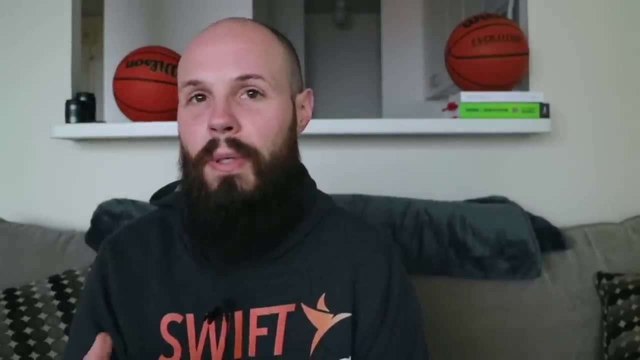 something from the ground up by myself is a huge confidence builder. Being able to accomplish something independently and figure things out on my own makes me feel like a real developer, And this was a major turning point in my career and my confidence, as well as when I built. 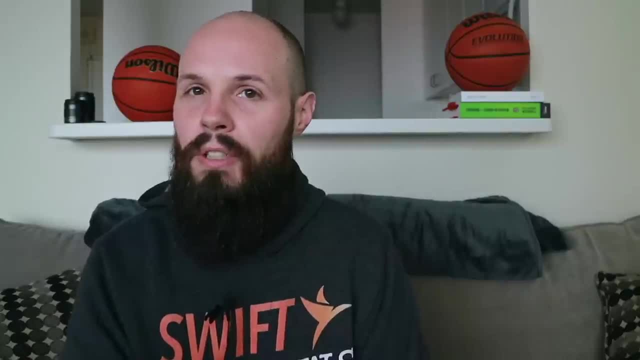 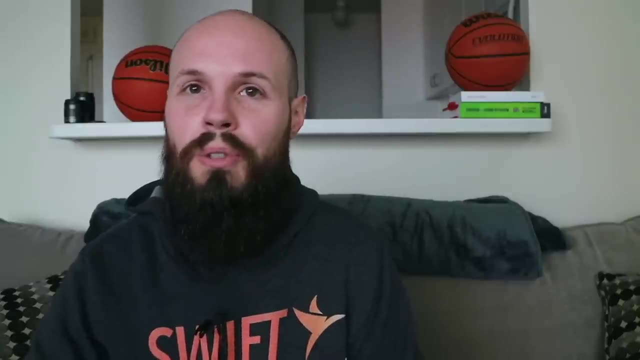 my first app On my own. I think what a lot of people can fall into, especially when they're just learning how to code or just getting started. you fall into what I call the tutorial trap, where all you do is just build tutorials, follow everybody's instructions. 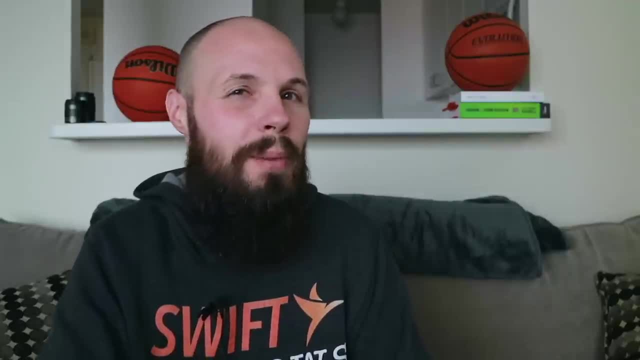 Sure, You've built three, four or five apps, but like they're not your apps, You just followed a recipe, so to speak, which don't get me wrong. You have to do that in the beginning, Like that's how you learn. 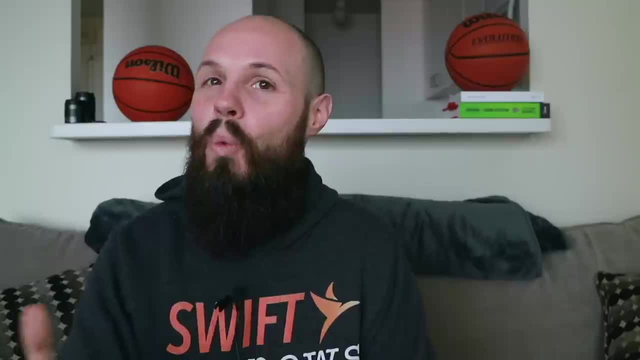 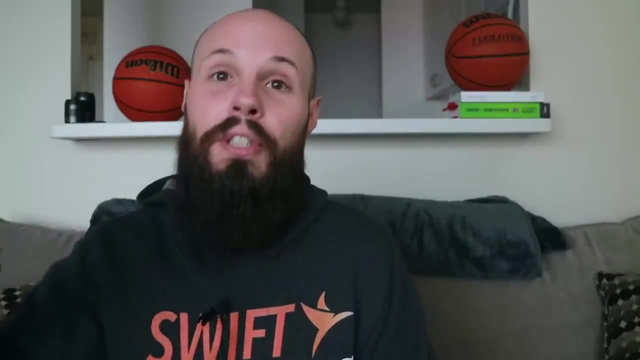 But what happens with people is they stay in that comfort zone way too long. And really what you should do to get out of that tutorial trap, Think of your own app. Think of your own idea and build it on your own. Build it yourself. 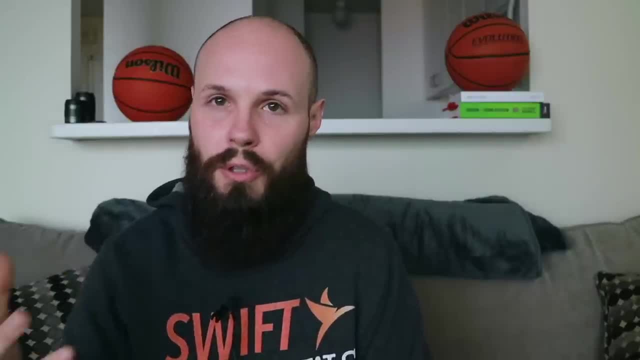 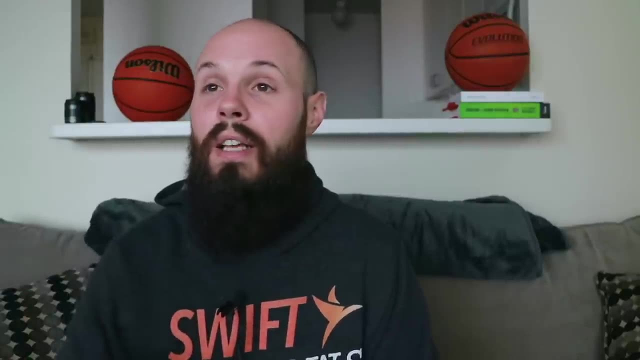 Don't get me wrong. You can look at references to help you build it, but you're not following the tutorial, You're building your own idea, And when I did that, I think my learning jumped up exponentially, because a lot of stuff I 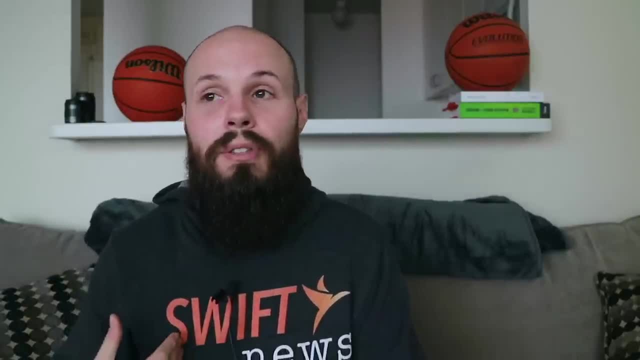 was doing. there wasn't a specific tutorial for, So what did I have to do? I had to dig into the documentation. I had to figure out and I'm not going to lie, It was hard as hell, Like it took forever. 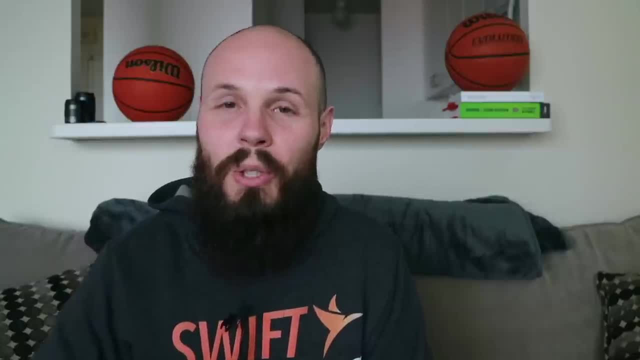 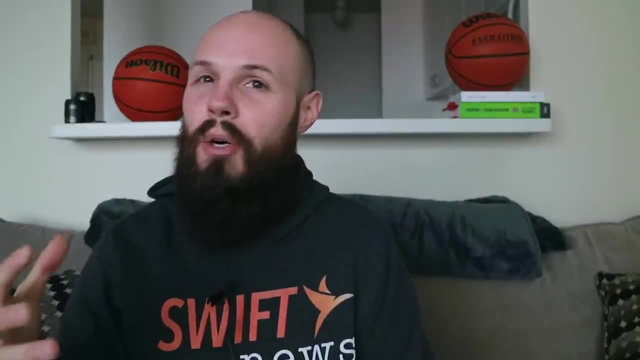 It took a long time, It was a struggle, but at the same time, I learned a ton doing it and when I got out through the other side, My confidence level was just high because, again, like I talked about earlier, I started learning how to learn, and that's just a huge thing. 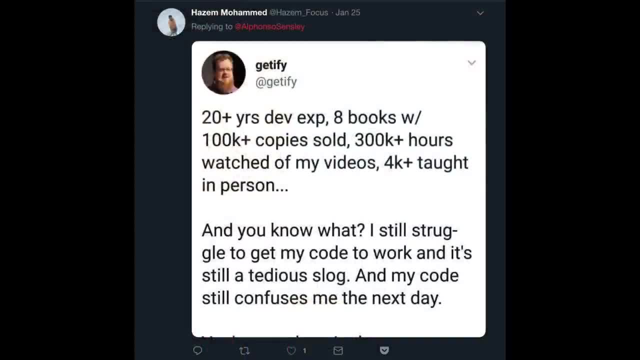 And then, finally, I want to end this on this. one from Getify says: you know, 20 plus years experience as a developer. He's got eight books with over 100,000 copies sold, 300 hours of videos watched, 4,000 people. 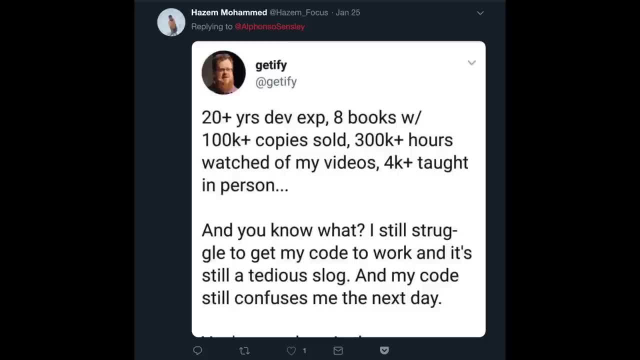 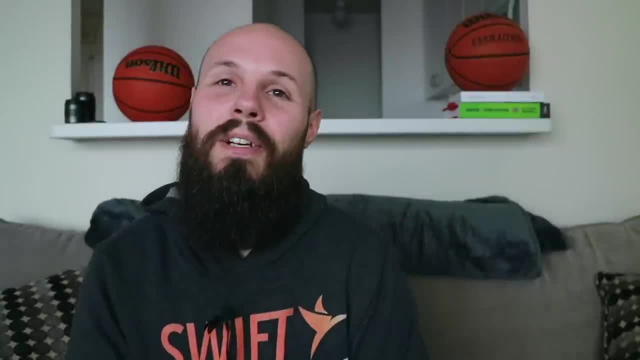 taught in person very accomplished developer right. And he says: and you know what, I still struggle to get my code to work and it's still a tedious log and my code still confuses me the next day. What are you saying here? 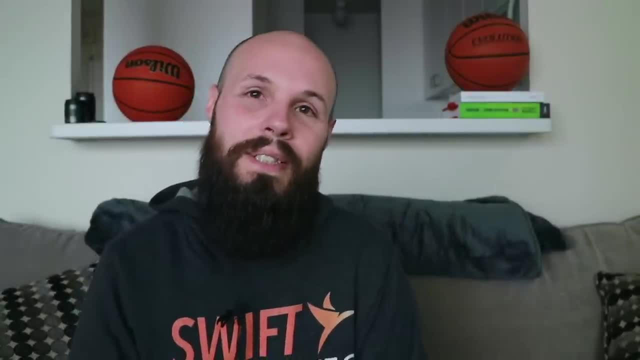 We all deal with this stuff. Like, no matter how experienced you are, you're going to deal with this, And I really like what he says, though, because it resonates with me. You know, I have 200 plus YouTube videos out there. 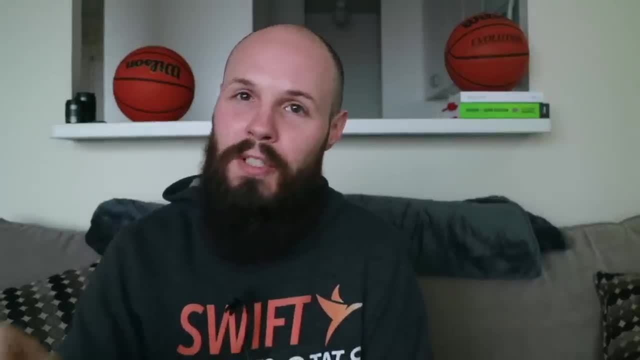 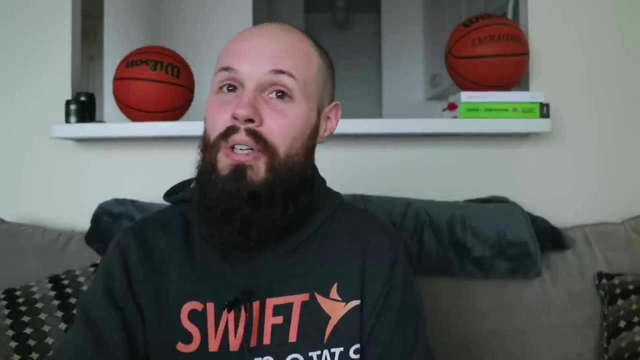 I can't tell you how many times I refer to my own video to implement something relatively simple, right? Because, like we mentioned earlier, it's impossible to memorize everything You're not going to know. But if you know where to look and know where to figure it out, you're good. 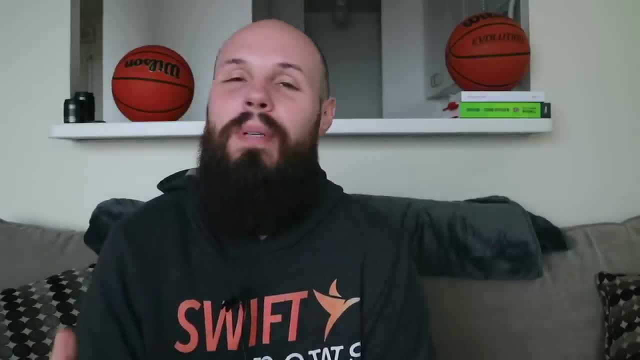 That's all I need to know. But again, the moral of this comment here is that just keep it in perspective. No matter how experienced you are, We all deal with this stuff, like the lack of confidence or, you know, confusing code. 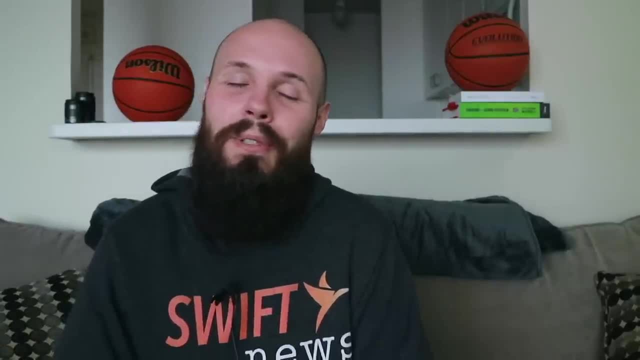 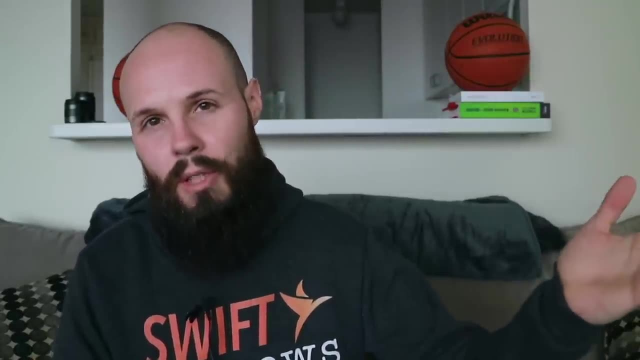 or having to look up the most simple things like: no matter how experienced you are, you still do that. So that's a few ways to build your confidence as a software developer. Thank you, Alfonso, for your tweet and, you know, letting me use that. 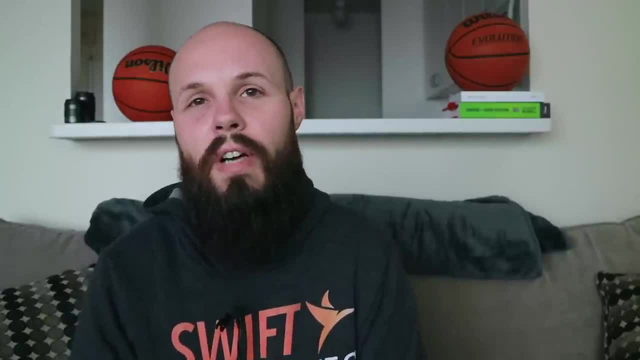 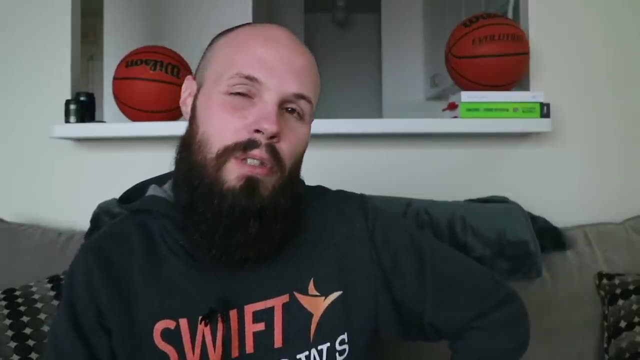 And then also anybody that responded in the comments. Great stuff, Very valuable Again. check out the tweet Link will be in the description, If you like what I'm doing here. I put out Swift news every Monday and a tutorial or two throughout the week. 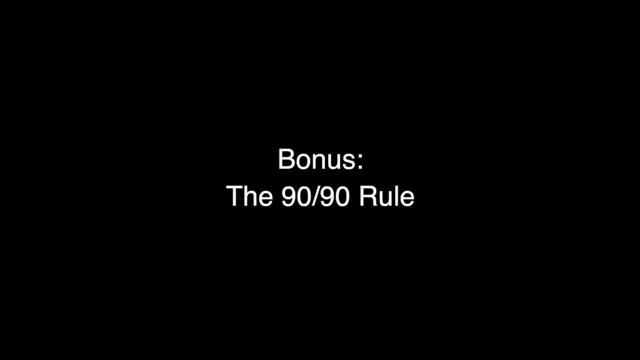 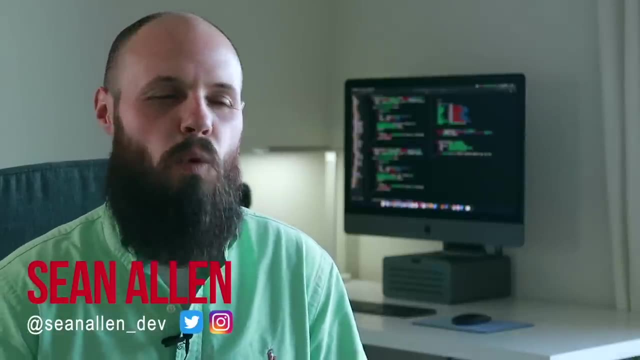 See you in the next one. What's going on everybody? Today we're going to talk about a software development concept that really only sinks in once you have experience, And there's not really an official name for it, but I call it the 90-90 rule. 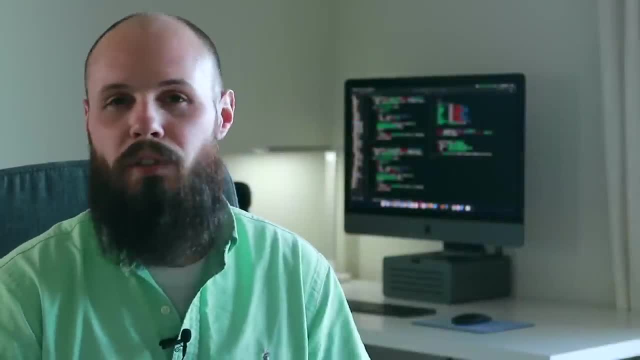 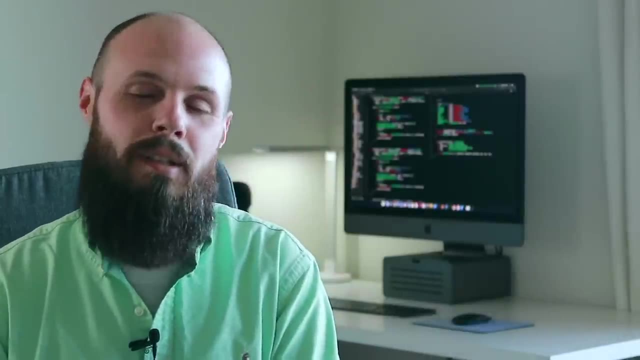 Now again. this will usually only bite you in the ass as a new developer, when you're building your first app or your first product, And that is the concept that there's the first 90% of the app and then there's the second 90% of the app. 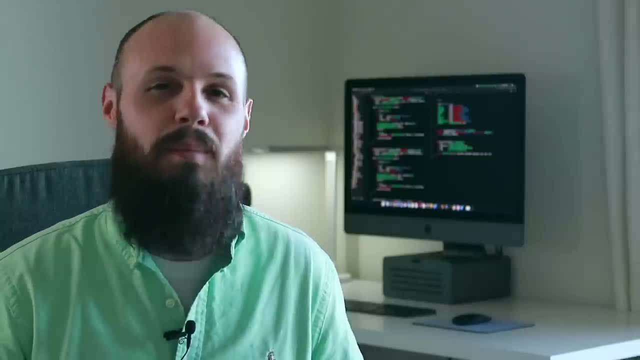 And you're thinking, wait a minute, 180%, what are you talking about? Like? what the hell does that mean? We'll talk about it. So here's typically what happens when you're building your first app, first website, first. 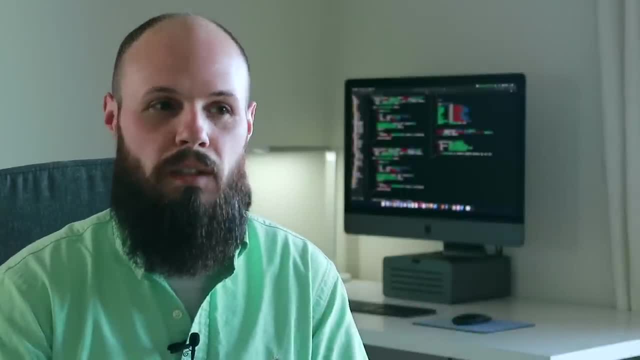 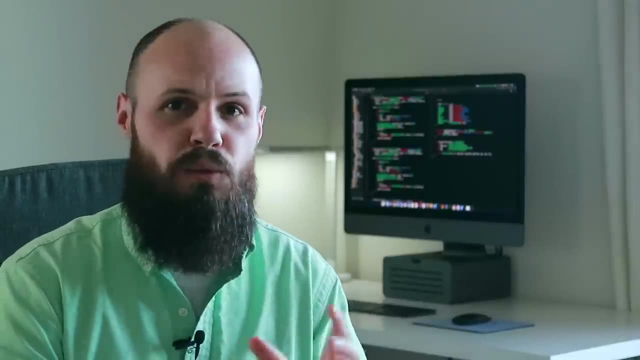 software development product. You're going to build that core functionality first. So when you have all that done, the app is going to feel like it's 90% done. You're going to be able to play with it, do all the main functions that you want and 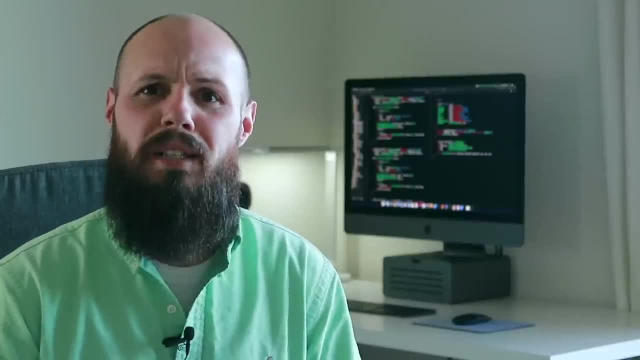 it's going to be like: wow, this app's ready to go almost. Just. you know, it's 90% done, just got a little bit of polish to go and we're done. Ship it. But that's where you'd be wrong. 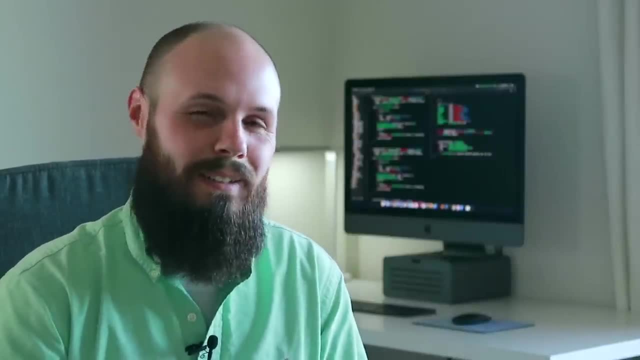 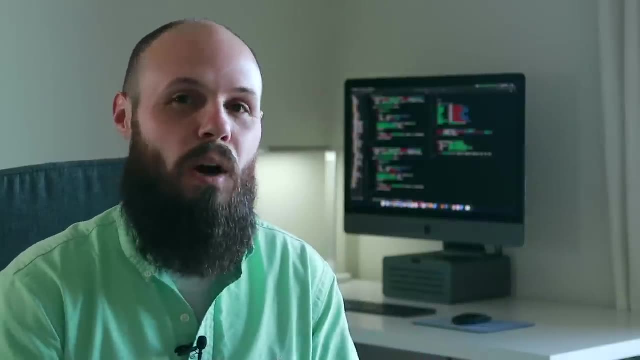 You see, that was just the first 90%, and even though it feels almost done, you're really only about halfway done. And that's where the second 90% comes in, And that's all this little stuff where each thing on its own doesn't really seem like. 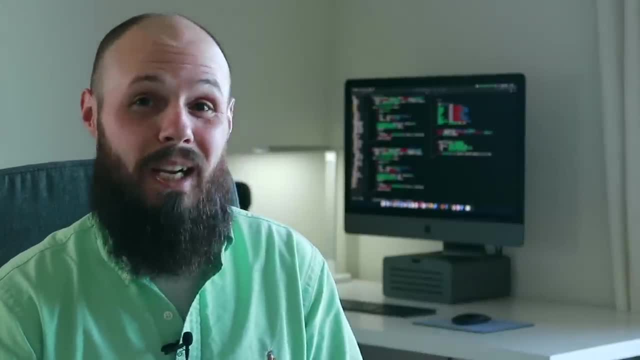 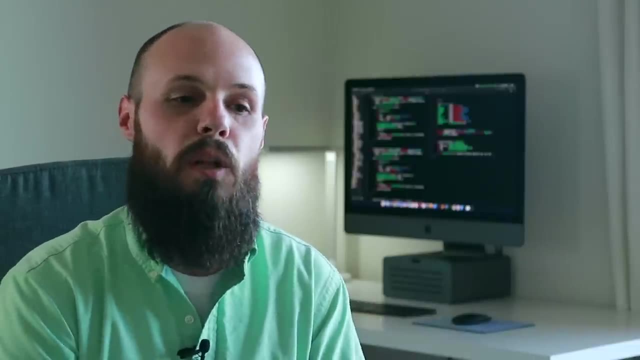 that big a deal, but they all add up to a lot of work actually, And that's why, when you get to that first 90% point, you're really only halfway done. And the reason I want to talk about this and bring this up to you, newer developers, is that 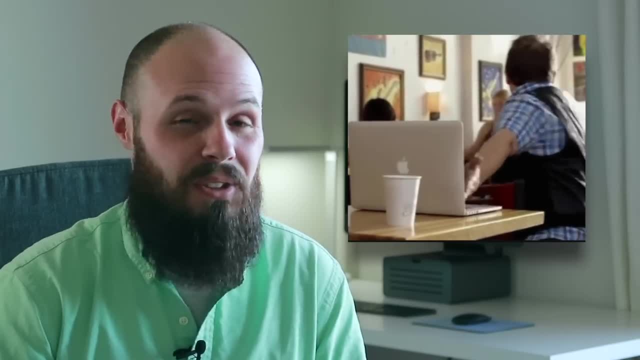 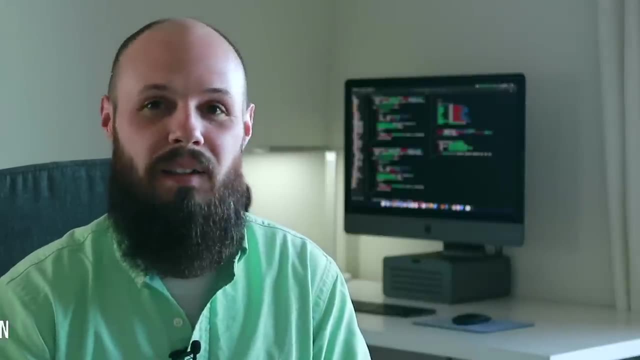 it can be very discouraging. I remember building my first app. It was discouraging as hell. It was frustrating, Like I again. I felt like I was almost done, This thing's ready to ship, And then it's just. all this little stuff just keeps piling up. 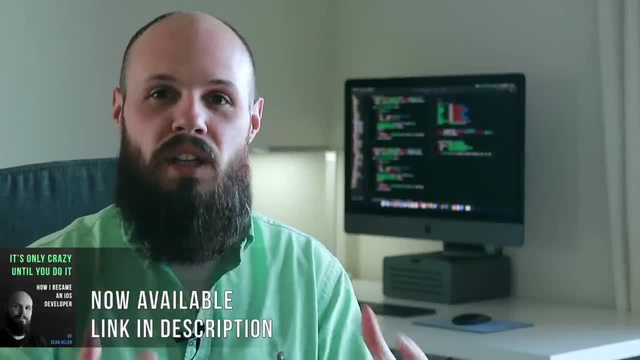 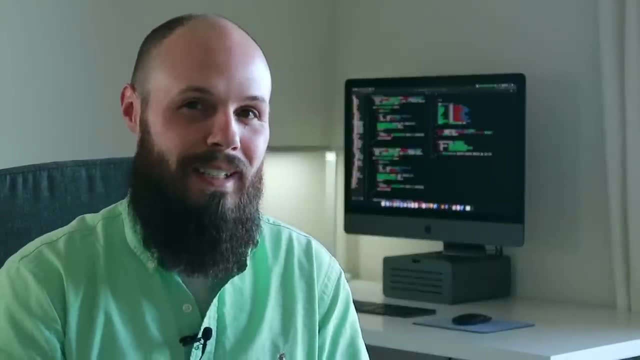 And we're going to talk about that little stuff later, But I wanted to share this concept, so you know this, going into building your first app, or if you're already midway through, you can kind of expect this, Because what happens is again: once you get that first 90% done, you think you're done. 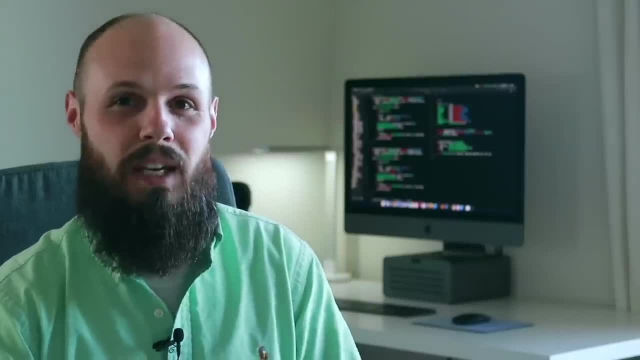 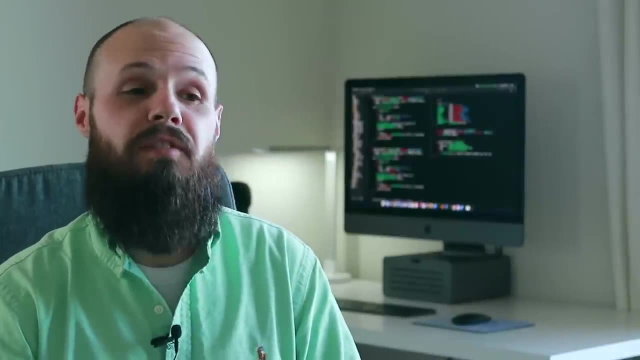 or close to being done, And then you just get smacked in the face by the second 90%. So I'm trying to forewarn you and let you know that second 90% is coming. So let's talk about that second 90%. that's about to smack you in the face. 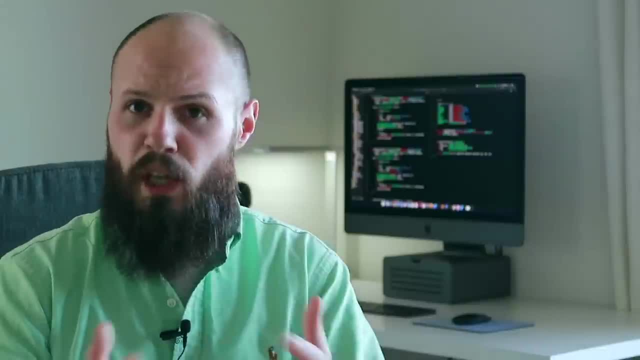 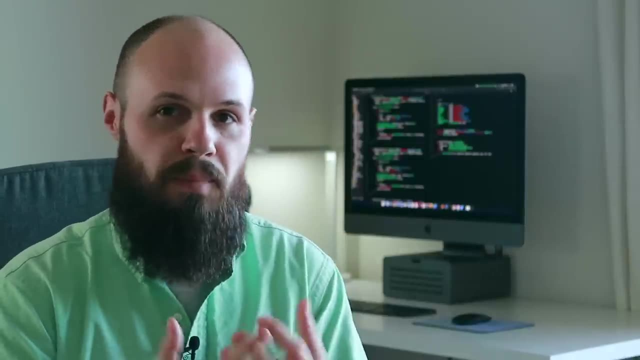 And we'll talk about some of the things that it can typically be. Now, if you're here watching this and you're not an iOS developer, That's what my channel focuses on is Swift and iOS development, So these examples are going to be from that perspective. 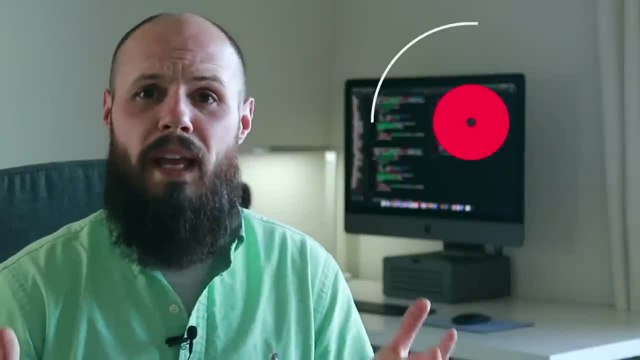 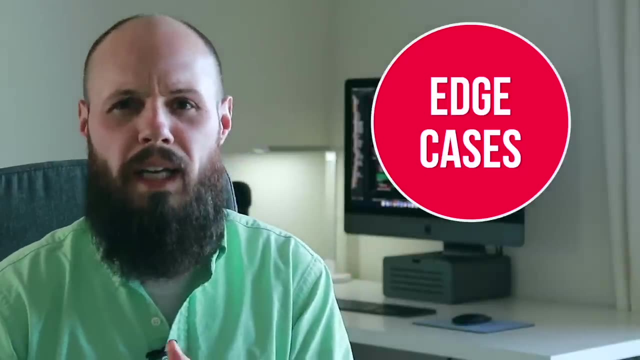 But you can apply it to your own process. But let's talk about edge cases here Now. this can be anything from: how does your app perform when there is no internet or very, very poor internet connection? You got to handle all of that. 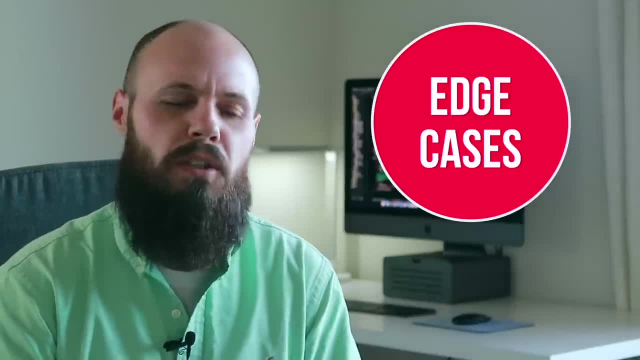 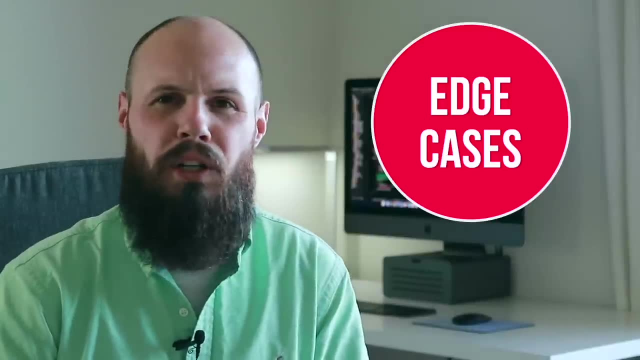 What happens when a user gets a brand new device? Are you relying on storing some stuff in user defaults too much? Or if they delete the app and reinstall, is your app still going to behave properly? Or things like what happens when a user kills your app? 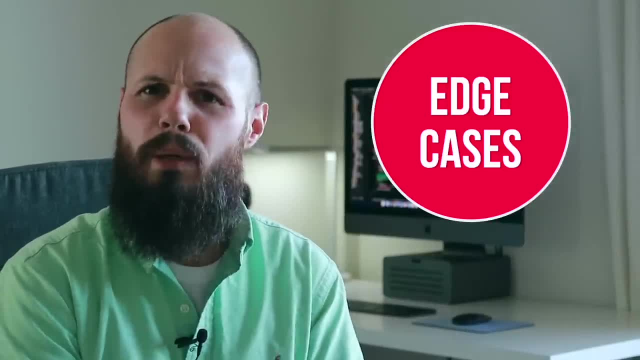 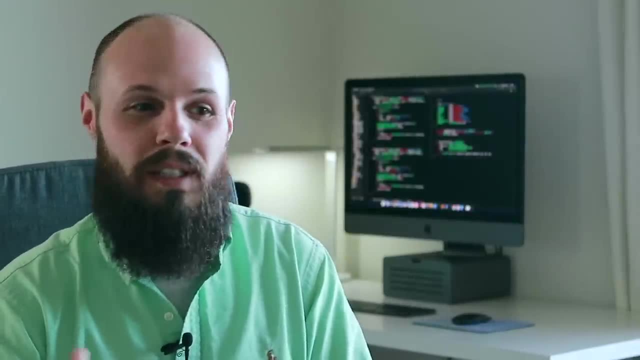 In the middle of a key function that's going on, Or is your app going to be able to recover from that, gracefully, Or is it just going to be in this weird state that's broken right. So you see, basically what really happens here is you think you know how users are going? 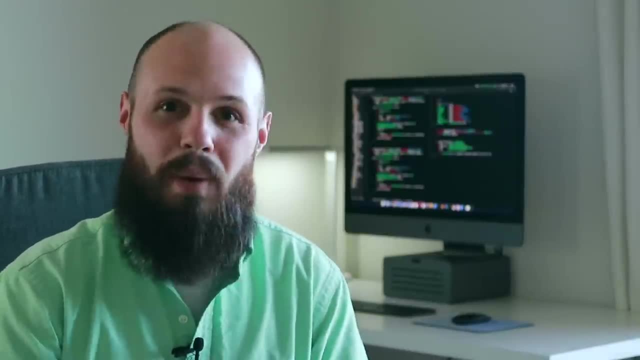 to use your app. But really, once it gets out in the wild and users start banging on your app, they're going to do things you could never, never even think of. So all these edge cases, you have to try and think of that in advance. 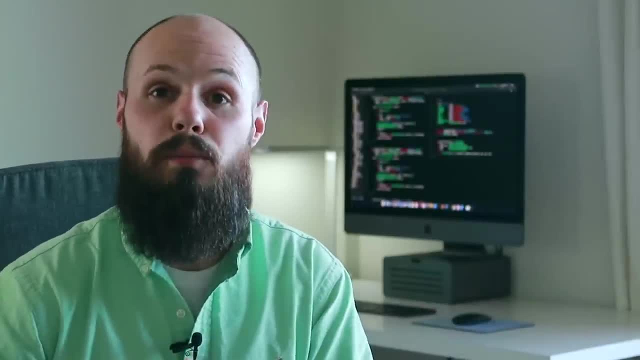 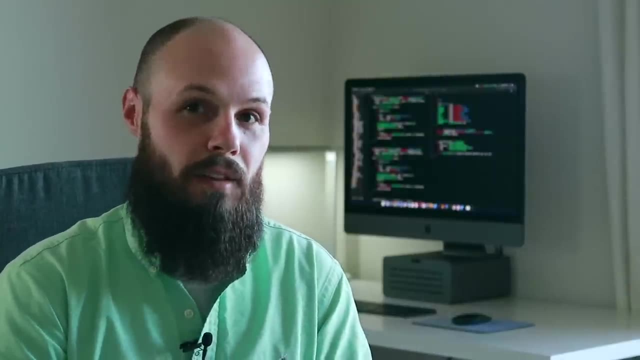 And, like I said, these small things really add up and do some time consuming fixes. And those were just some common, general edge cases. You know these edge cases are going to be very specific to your app, but they really add up. Next up, let's talk about some really robust error handling right. 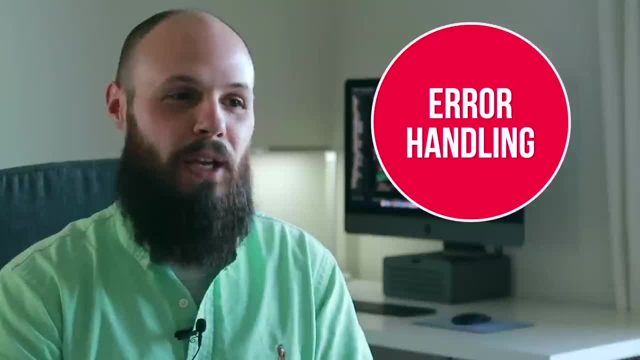 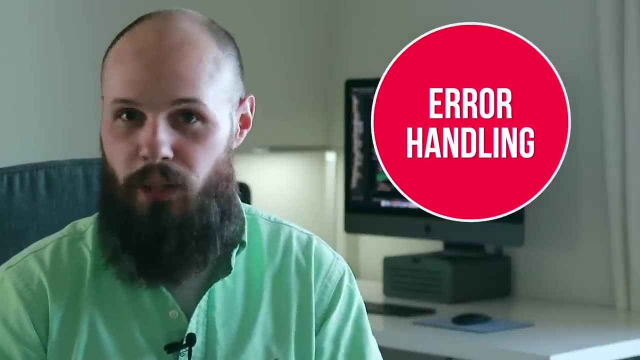 When we're initially developing our app. how common is it to be like to do? handle the errors, and you'll do that later. right, Because it's tedious work, because you've got to handle all the various different error messages and fail gracefully like we do in our apps, right? 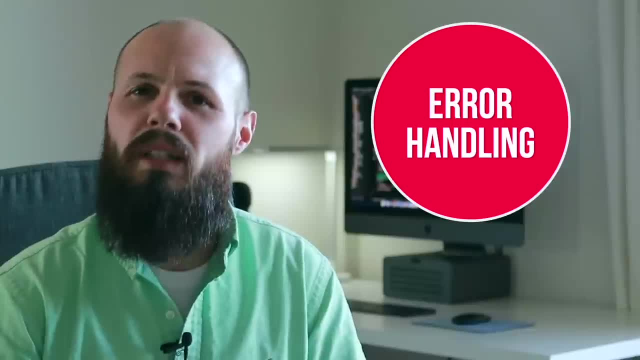 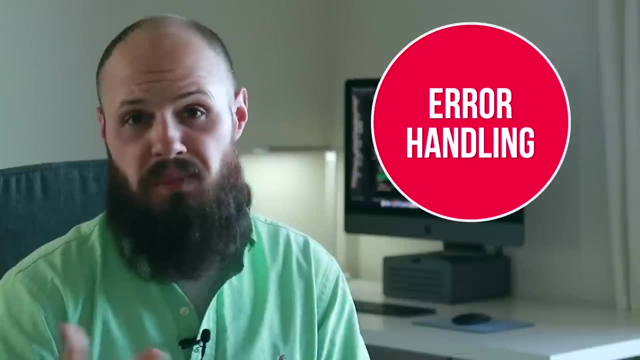 You don't want to just have an abrupt error that's not descriptive, you know. you want to let the user know what's going on so they know what happened with your app and so forth. So building out really robust error handling. It's tedious and time consuming, but it has to be done. 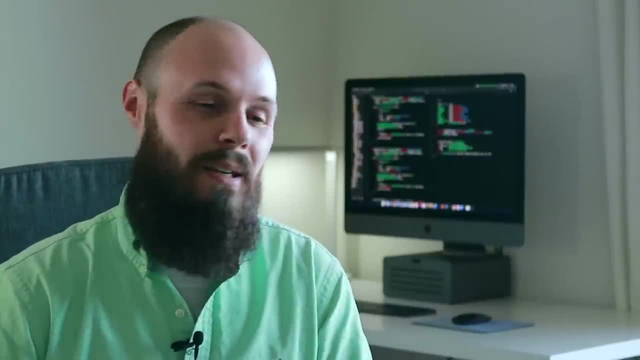 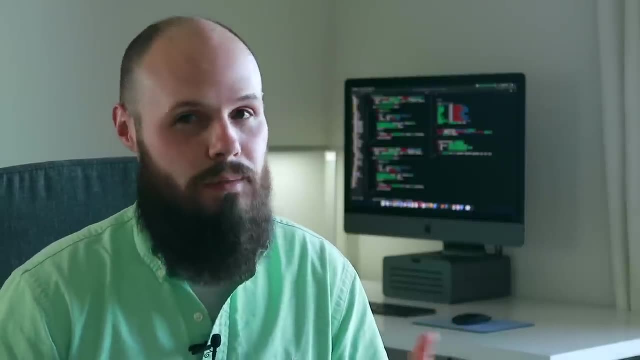 And again, it's one of those things where on its own may not seem that bad, but when you pile on error handling with edge cases and all the other stuff we're going to talk about again, you can start to see where this second 90% again it adds up, you know, and 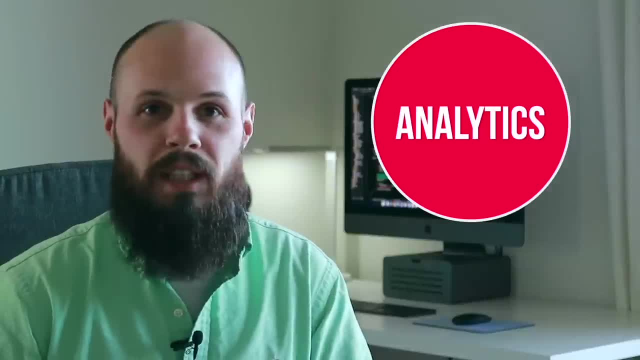 then you have things like just overall analytics, right? You want to see how many times users are going to a specific screen or how many times they're doing a specific function. So now you got to. once the app's done, you got to, you know, put in your analytics. so 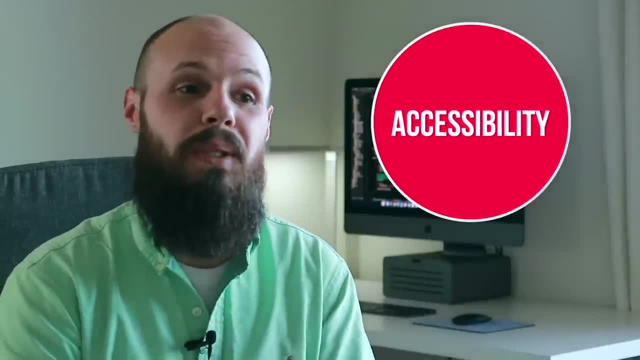 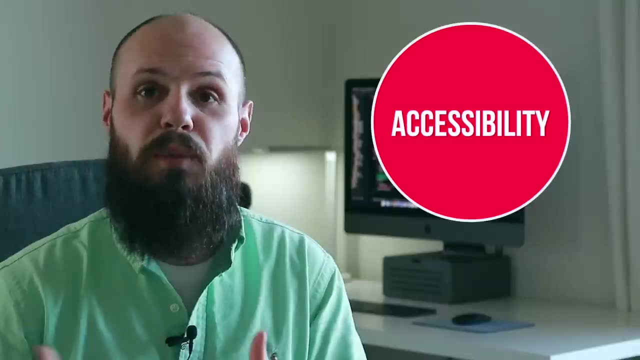 you can track everything. And then there's accessibility features for people with disabilities, And This is often overlooked by many developers, but it's so, so important. I've covered it on Swift News a few times. Just the percentage of people that you know use the iPhone that actually use these accessibility. 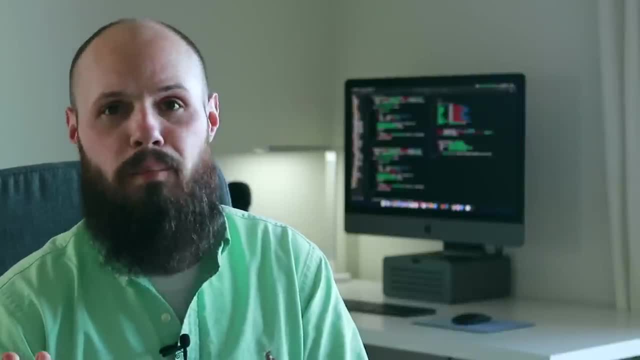 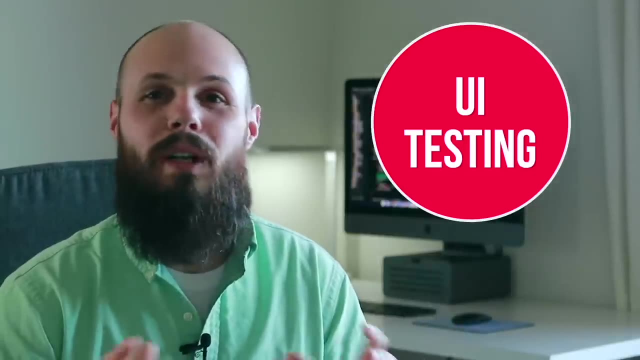 features. It's a big deal. And if you're ignoring accessibility, stop, you shouldn't. And then you got testing your UI on all the many, many device sizes here in the iOS ecosystem. Now don't get me wrong: If you're using auto layout correctly, that's going to handle 80 to 90% of the work in my 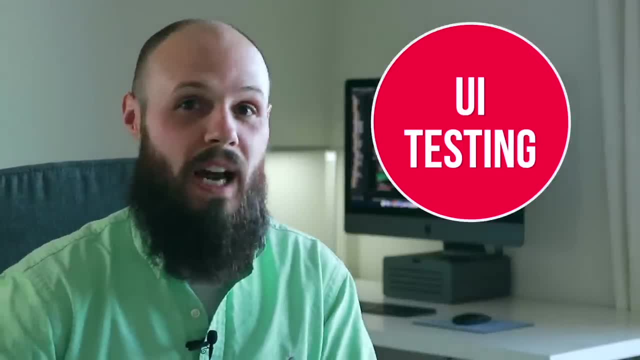 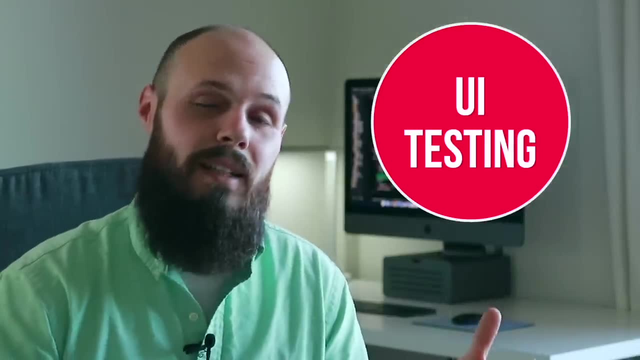 opinion. However, you know, making your app look beautiful on the iPhone XS Max- Yes, I said XS- And then down to the iPhone SE size like that's a massive difference And, like I said a lot of times, auto layout will do most of the work, but most of the 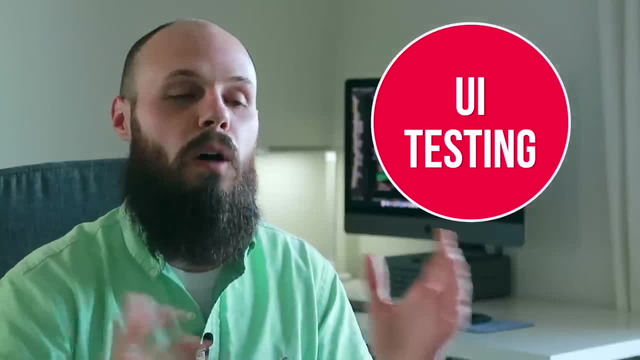 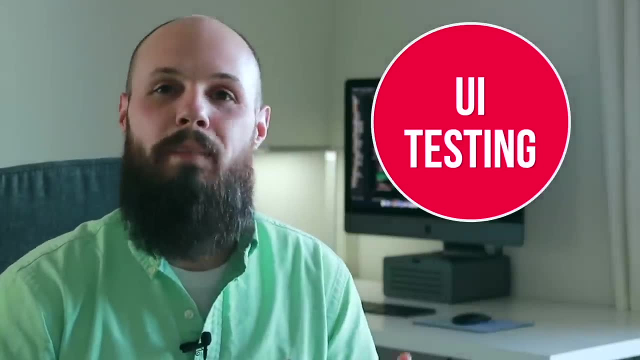 time you got to tweak that final 10% to get it really looking perfect on both screens. And, like I said in the beginning, when you're building the original functionality of your app going through the first time, you're not worried about making it look great on. 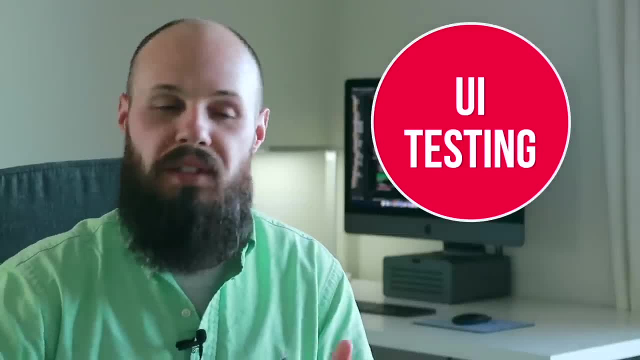 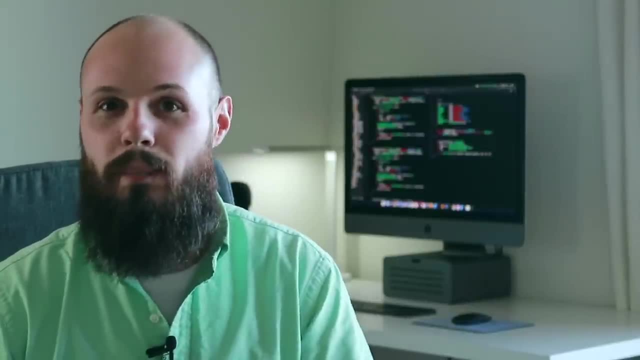 all screen sizes while you're still building it and trying to get it to work right. You kind of save that for the end, once you're ready for the polish. But again, now we're just piling more stuff up Up onto that second 90% that we're talking about. and then there's the good old refactoring. 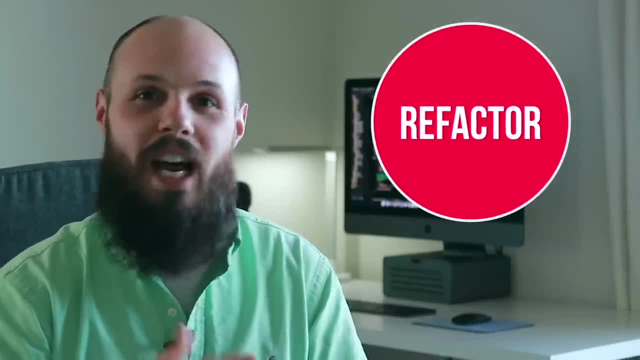 How many times have you built a feature? you know to do refactor this later when you have more time right? Because oftentimes in software development you, you just hack it together to get it working and then you clean it up later.